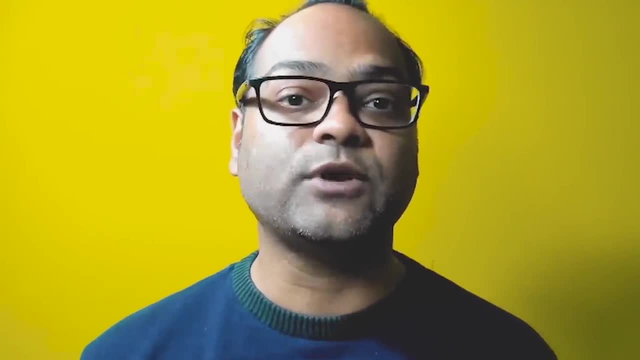 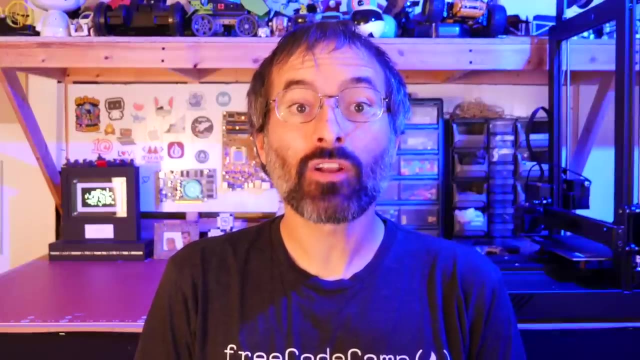 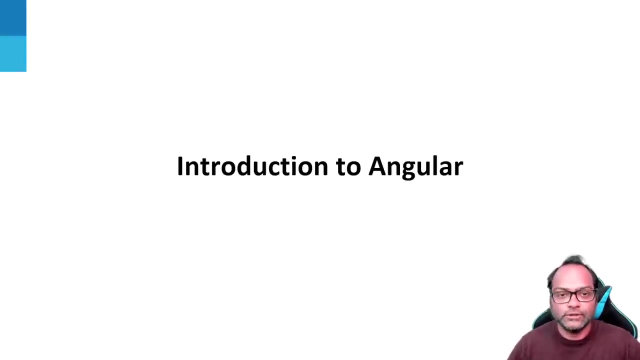 for this course. He is a Google Developer Expert for Angular, a GitHub star and an active contributor to both Angular and NGRX, So he is the perfect person to teach you Angular. Hi, welcome to this course on Angular Getting Started. In this video we are going to introduce 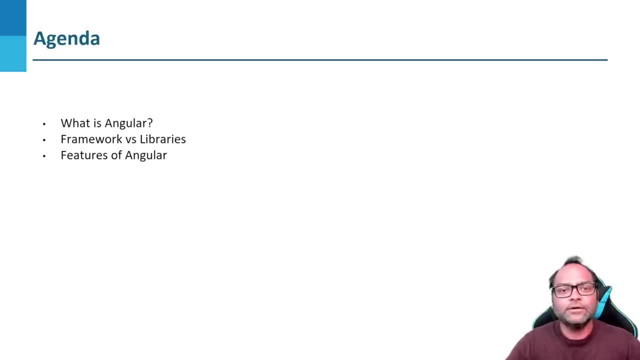 Angular. So we will talk about what is Angular. We'll talk about framework versus libraries and at the end, we will see some of the features of Angular. So we'll see a tiny to-do app and we'll go through some features. So let's go through what is Angular, which is really. 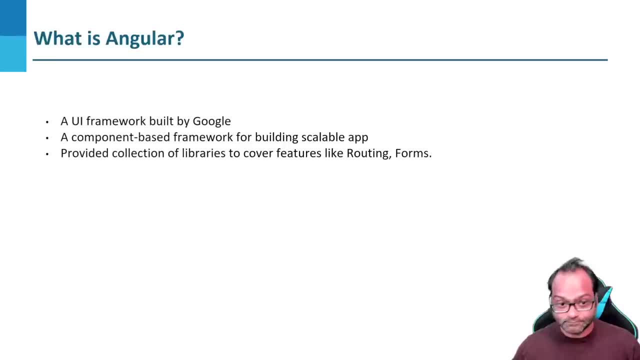 important before you go ahead and choose Angular as your framework. So Angular is actually a UI framework built for Angular. It is built by Google and it is actively maintained by a team within Google, which is the Angular team, And it has like around 30 members who are actively working on it. 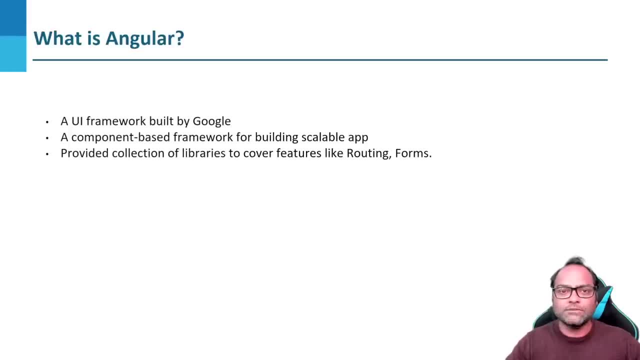 Angular had a previous version, So there are some confusion regarding that, So let me just clear it. There was a framework called AngularJS- I'm saying was because it will just reach its end of life- It was created back in 2009, and it was created using JavaScript, So it 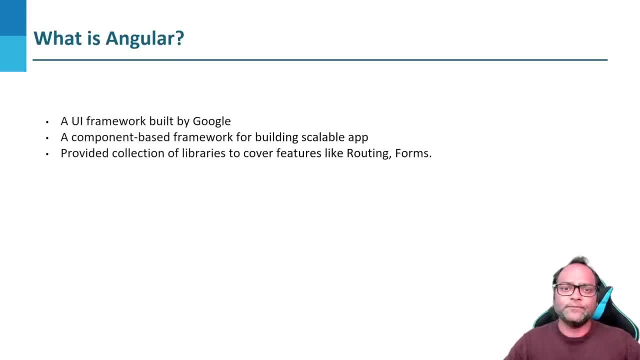 was a framework that was created in 2009.. So it was created using JavaScript. So it was created using JavaScript. So it was created using JavaScript. So it was created using pure JavaScript. framework Around 2014,. Angular team decided that they will be rewriting. 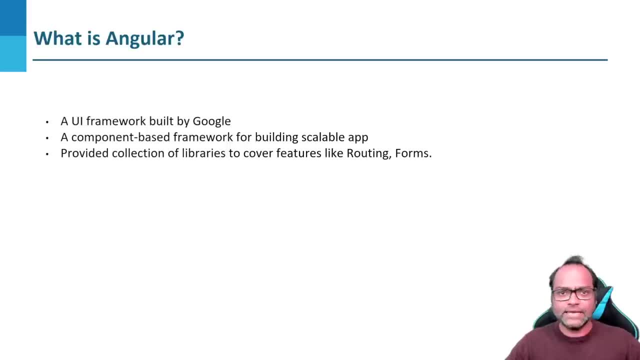 the framework and they'll be creating a new framework. They initially named it as Angular v2.0. But later they decided to drop that v2.0.. They said: it's Angular, So we have AngularJS, and now we have AngularJS. and now we have Angular, That's it. And so, after the initial 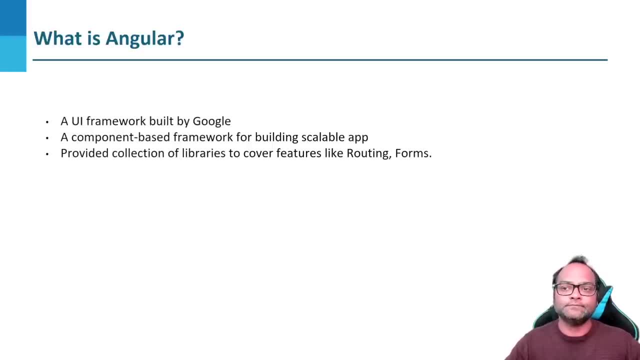 release of Angular. They decided to set a release cycle for the framework. So every six months there will be some new additions, new feature requests, new enhancements, some bug fixes which will be released. So it happens every six months. At the time of recording this video, Angular. 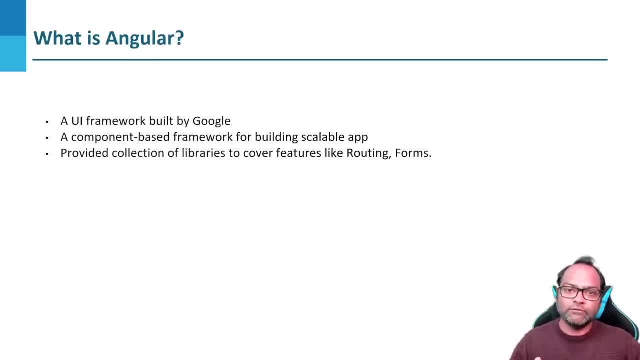 version 13 just released. So, if you are wondering, we will be using v13 for this particular course. no, because we want the stable version, So we'll be going with Angular v12.. But at the end we can actually provide a video which will walk you through how you can upgrade. 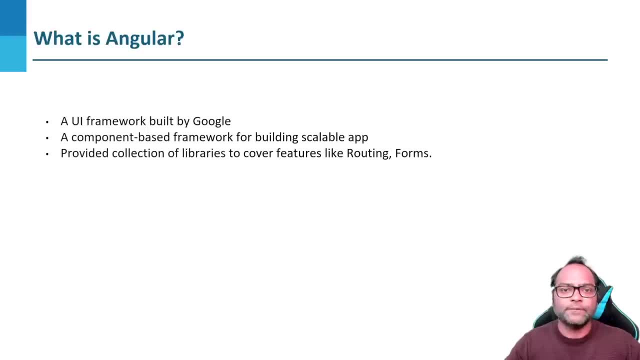 from Angular v12 to v13. So that will be covered. So that's about the framework And one important thing: when the Angular team decided to rewrite the framework, they chose TypeScript as the language to rewrite the framework. We will go through TypeScript in upcoming videos. 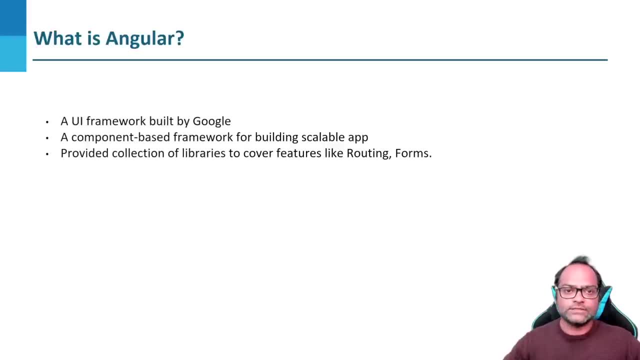 So we'll talk more about it here. What else? Angular is a component-based framework for building scalable apps, So it's almost first choice for all the enterprise applications because they want to release faster, which you will see in this course. Once we start implementing new features, you will see how. 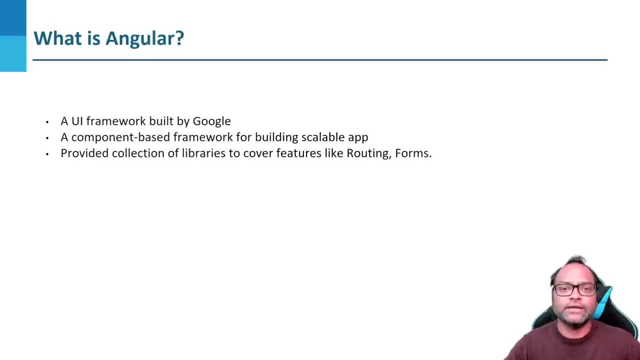 fast we can actually do and deliver things. So that's why it has been the number one choice. So if you're thinking about what's component, of course we are going to talk about component. There will be an entire section which will talk about it. But just let me tell you a. 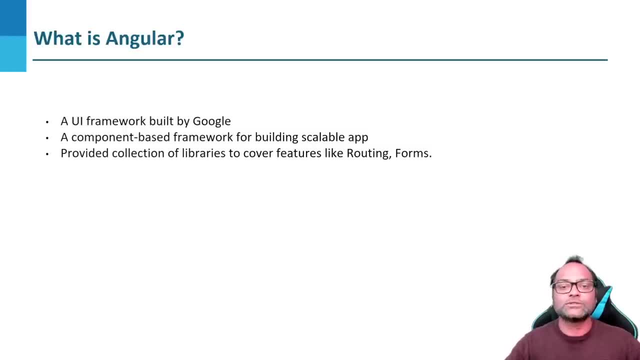 little bit about Angular. Let's talk about what component-based is. So you use a lot of websites in your daily life, So you might have visited, let's say, if you are trying to learn Angular, you might have visited angulario. or let's say, you. 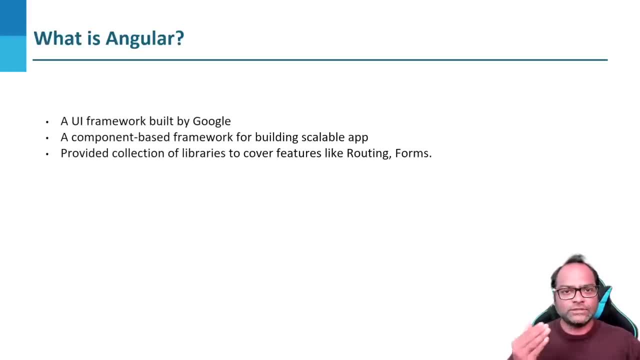 use Facebook, Twitter every day. So if I have to tell you what components are on those websites, so you might have seen there is a sidebar, there is a header, there is a footer and there are some content areas. So, for example, in Facebook you will see cards On Twitter, 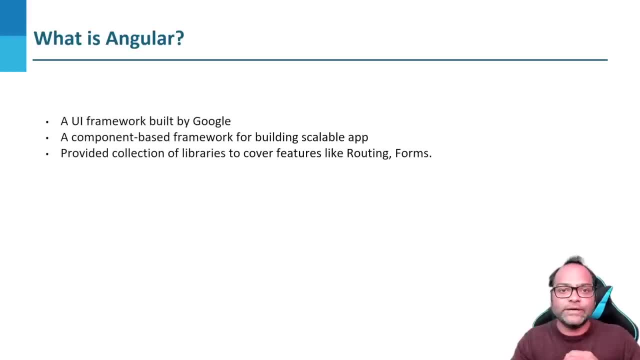 it's totally different. So those are small components. And all the frameworks which are out there- for example, React, Vuejs, Angular- they're all component-based, So you can create components and then you can build small, small components. 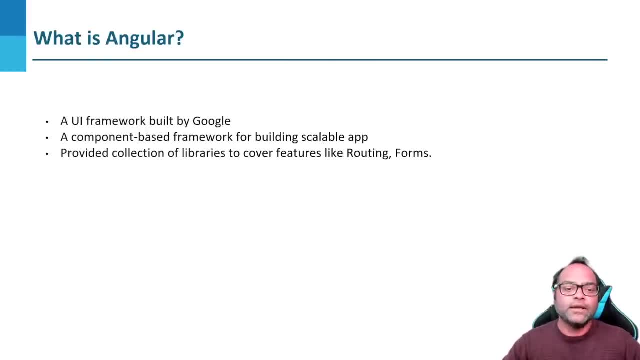 and attach them together and build your application. Angular being a framework, it provides you a set of libraries and it has a lot of features included as part of the framework. So you have routing, you have forms, you have PWAs and many more. 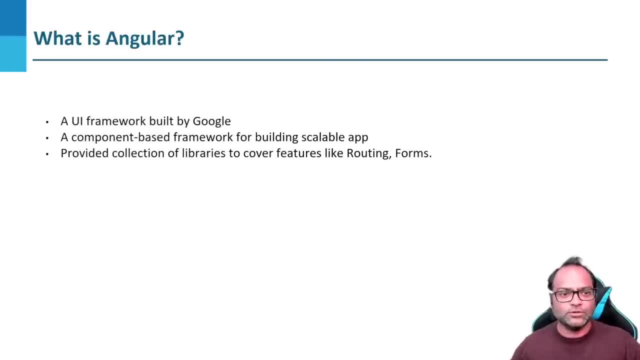 So you have data binding. So we'll talk about those features. Let's talk about framework versus libraries. What is framework? So frameworks really contains a set of libraries. So what I mean by that you might have used, for example, in case 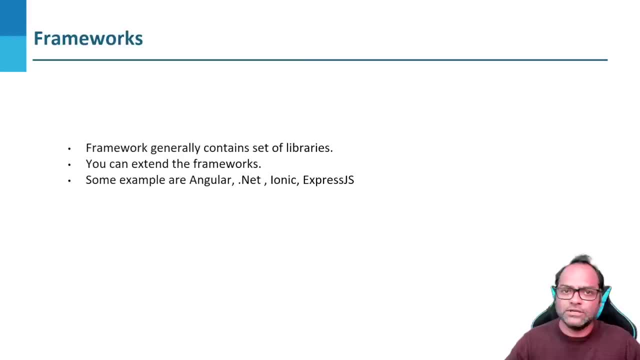 you have never used it, that's absolutely fine. But in case you have used some technologies like Java NET in the past, you may have seen we use something called using or we do something called import in Java. So what do you do? 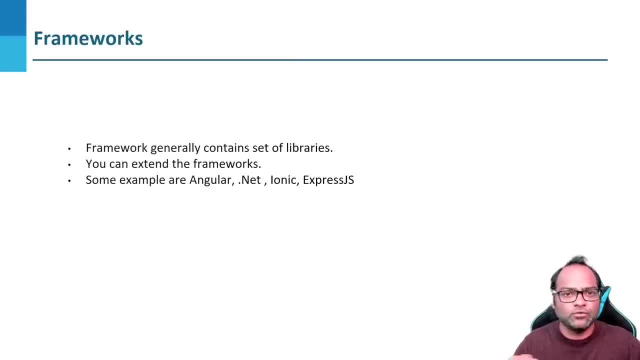 You actually require, or in case you have written, let's say, Nodejs code you may have seen require, or now the latest version support ESM, so you might have used import. So what we do? we actually import some libraries. So if I talk about frameworks, those libraries. 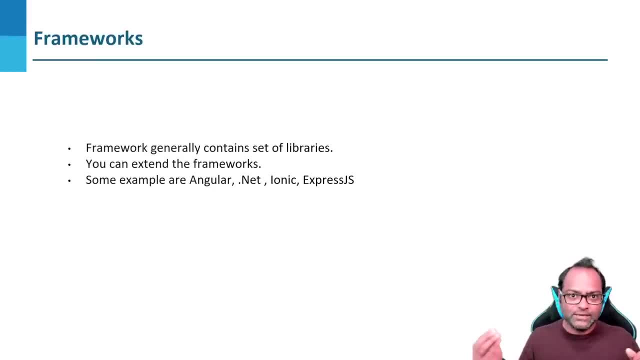 are part of your framework itself, for example in NET. So all the namespaces which you import or you use are part of the framework itself. You don't go outside. Similarly, in Angular framework also, you have a lot of features. For example, let's say: let's say: let's say: 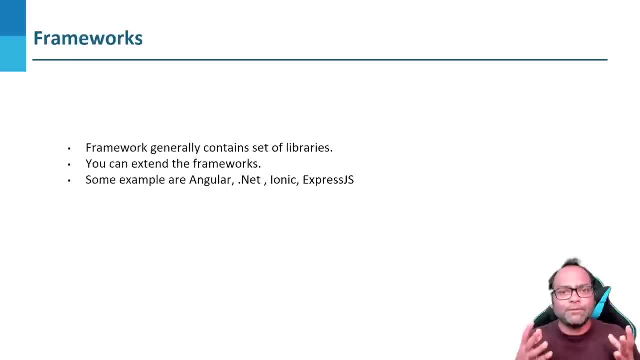 I spoke about routing forms. Those are part of the framework, So you can just import it from the framework itself. You can extend the framework. of course, You can build something on top of your framework. INX DevTools is a good example. You have INX Framework also, which uses some of the features. 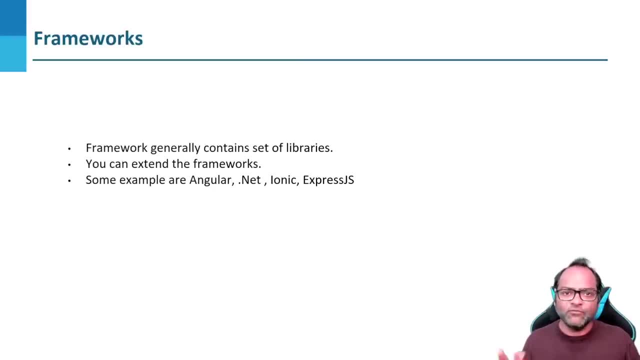 provided by Angular. So, as we said, there are some examples of frameworks. You have AngularNET, You have Java, You have INX Express, You have JS. So those are some examples. Now let's talk about libraries. So libraries, when we talk about libraries, we talk about some specific functionality. 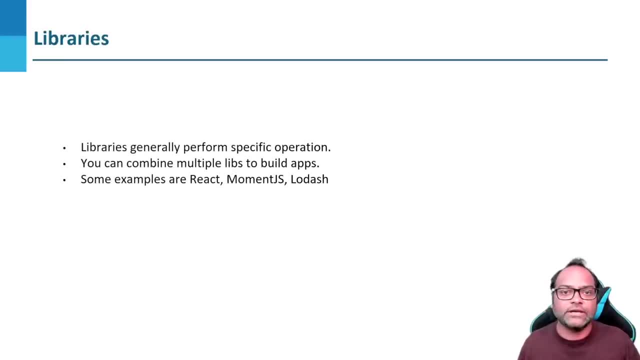 For example, let's say, if I have to use Lodash, which is a really good library out there. So what Lodash contains? Lodash contains a lot of utilities, functions which you can use to avoid a lot of code in your existing code base. So if I have to compare to objects, 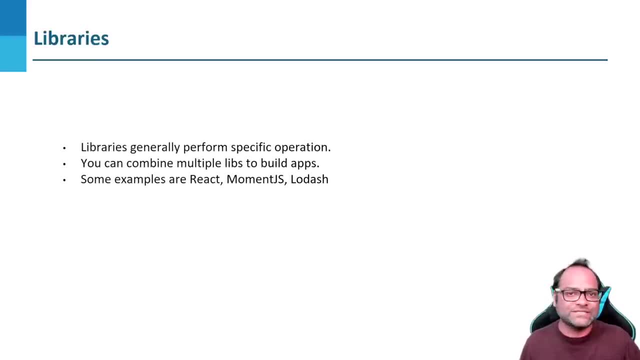 I can just import something or use something from Lodash rather than adding my own, So you can actually combine multiple libraries, For example. let me take an example of React, in case you know about React, So in case you want to create an application using React. so what you will do, you will. 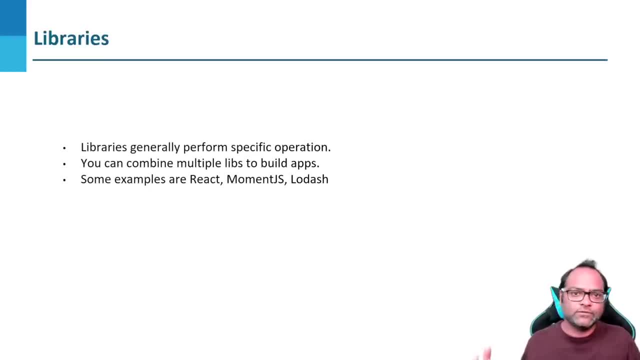 take React, You will take React Router, You will take some of the Form library which is available which suits your requirements. So you will combine all those libraries and build your application. That's what you do, So that's libraries. So some examples: of course, React, MomentJS- MomentJS has been deprecated, but yeah, it's. 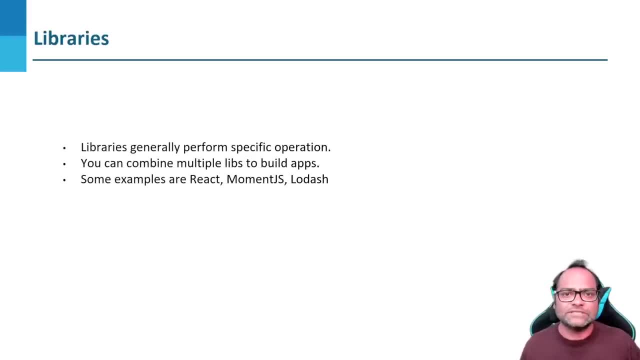 a date time library. Now you can use DateFNS, which is a replacement for MomentJS, and you have Lodash. Let's talk about some of the features which is available. We are not actually going to go into detail, because we are going to go into more detail in the upcoming videos. 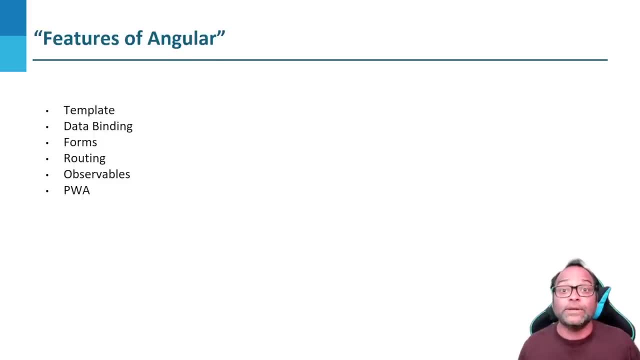 So there are a few features which is provided by Angular. For example, it has its own template engine. It provides you data binding, so you can bind the data on your front end. It has forms routing. It provides you observables, which is actually another library, but heavily used. 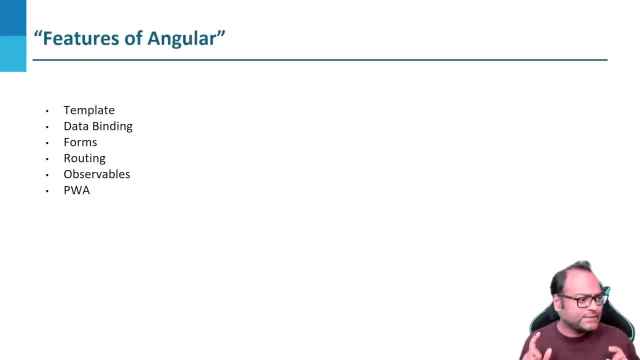 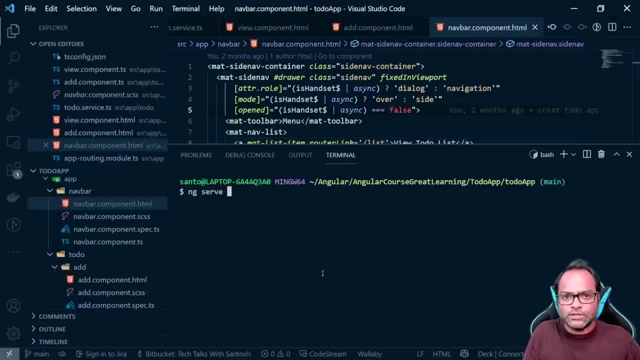 inside Angular and PWS, right. So let's see an app. So it's a small to-do app. Don't worry about the command as of now. So I'll start this to-do app and we will see some of the features in action. 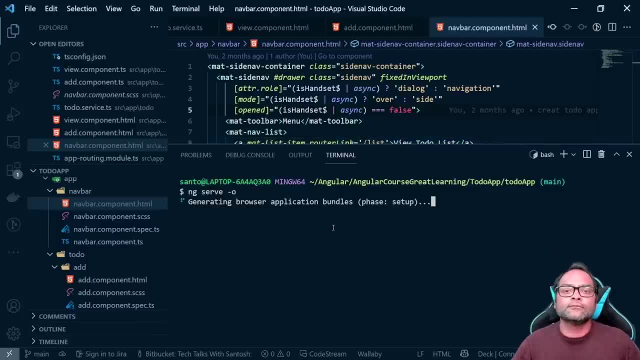 You will notice, it's an exclusive to-do app, So if you haven't looked at it yet, you will notice the link for the lessons, learning meetings series is over here. So that is it And here. we just showed it on the screen because we will see some new features related to it. 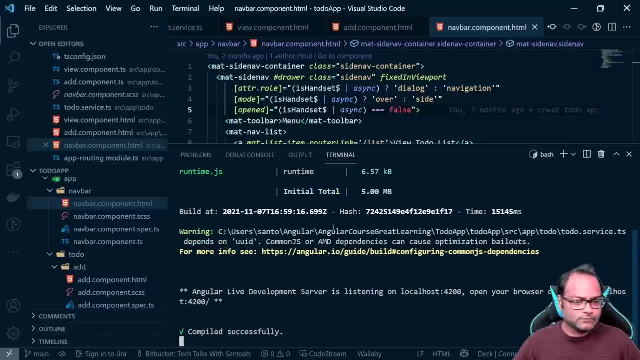 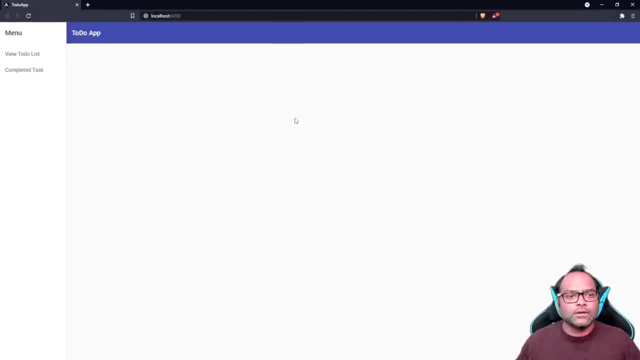 So phase-1 is added. we have the integration. let me open the video and you can see it actually looks like everything is on the screen And basically we can see. Sorry, Let me open the video page And then after that you can do all the changes and do some modifications as needed. 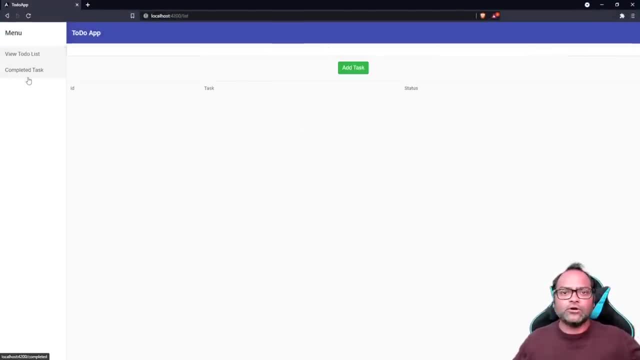 app. so you can see i'm whenever i click on this url, so i'm actually being redirected to another url. so this is routing. so this is routing functionality. you can see, this is a form where i can input some values. so let's add pay bills as a task or buy groceries as another task. 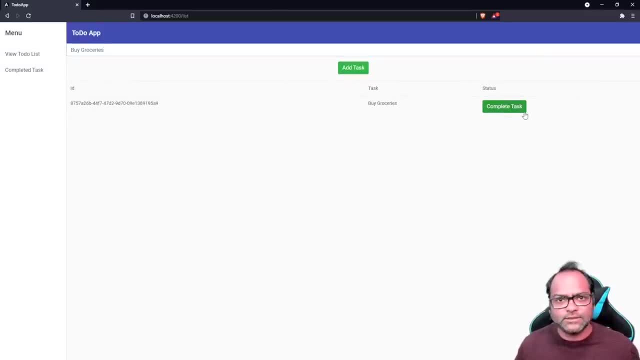 so these are two tasks which i've added. now i can also mark this task as complete, so, and then i can go to completed task and see what are the tasks which are which has been completed. so what we have seen here is: you have data binding functionality, you have forms. 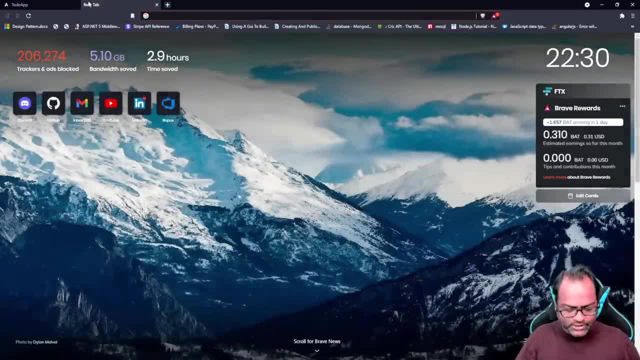 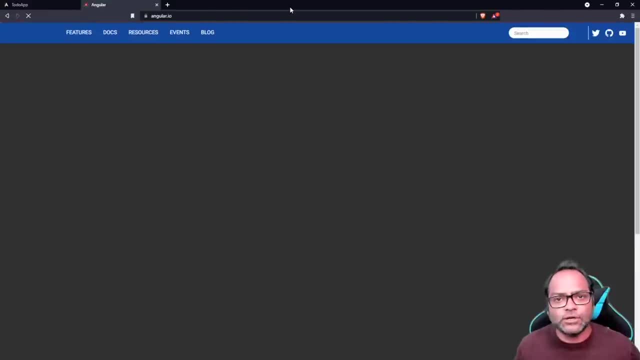 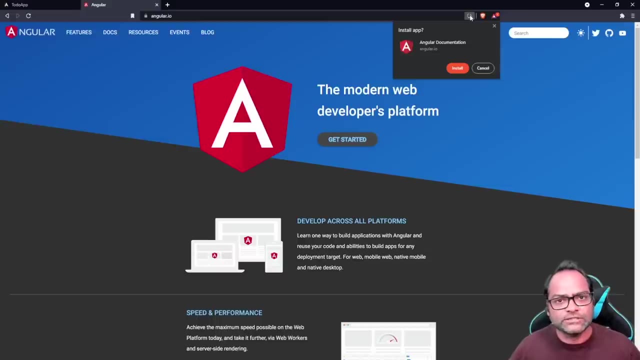 you have routing. let me show you pwa as well, because it's being talked about a lot, and let's see what actually pw is. so whenever you visit some website, you might have seen this symbol. it says install app. this is pwa functionality. so what you can do is 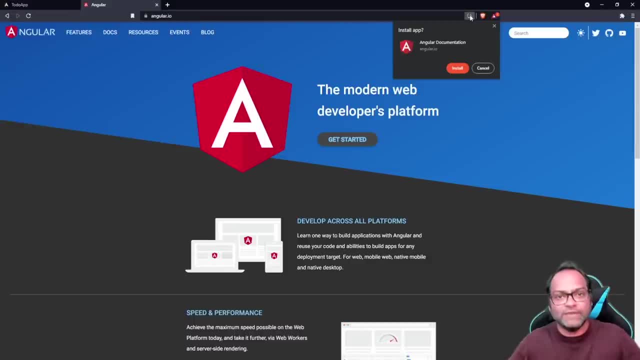 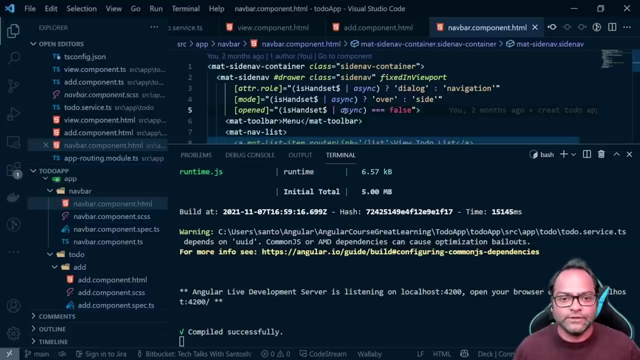 you can install your website as a native app, it will behave like a native app in case you install it on your mobile. in case i install it on desktop, it will behave like a desktop app. so that's, that's about pwa. so that's it from this particular video and we'll move to the next video now. 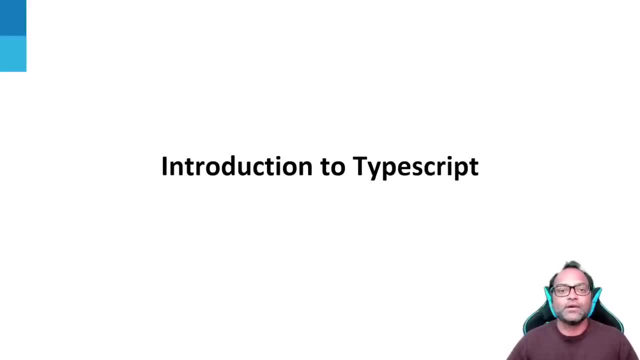 hi, in this video we will talk about typescript. as we said in previous video while introducing angular, that typescript is a language in which the entire framework is written and we need to write our code in typescript as well. so we are going to go through, of course, we will introduce you to typescript. 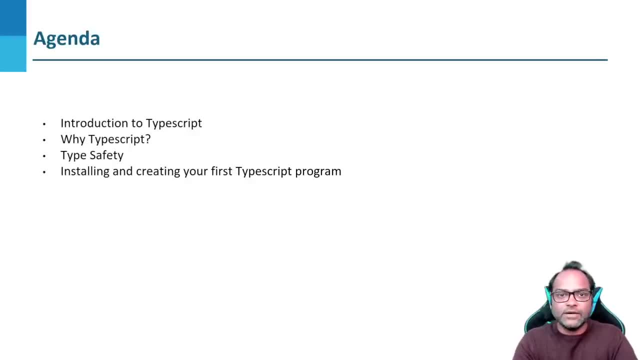 we'll talk about some basics, i mean, how the language came and who invented it, and then we'll talk about why should you learn typescript, of course, the one reason being you have to write your angular code using typescript. but yes, there is more. then we'll talk about type safety and at the end we will see. 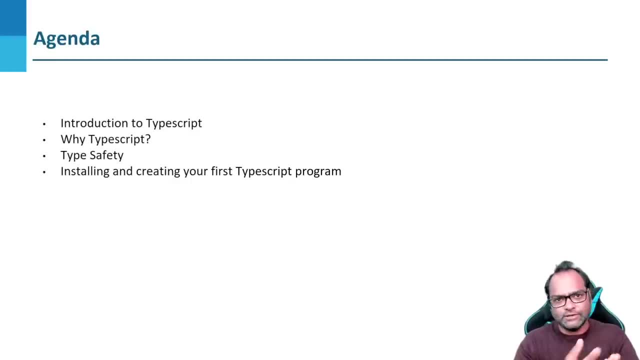 we'll install typescript and then we'll also write our first code and we'll execute that code. so let's go ahead and get started. so what is that? what is the typescript, right? so let's talk about that first. so it's a strongly typed programming language. now you might be wondering what is. 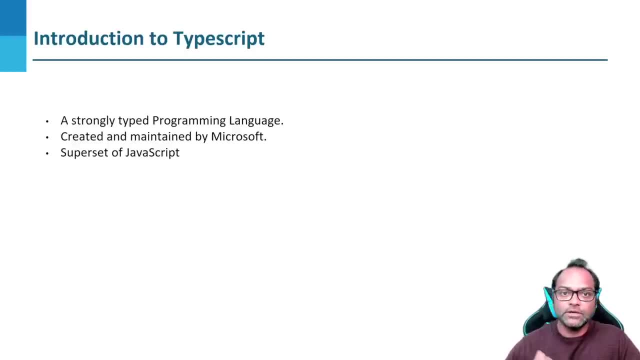 strongly typed programming language. so in case you are new to typescript, just hang on. we will be talking about it in more detail. but in case you are coming from languages like java or dotnet, or in case you learned the java or dotnet in past, so you might have seen that whenever you declare, 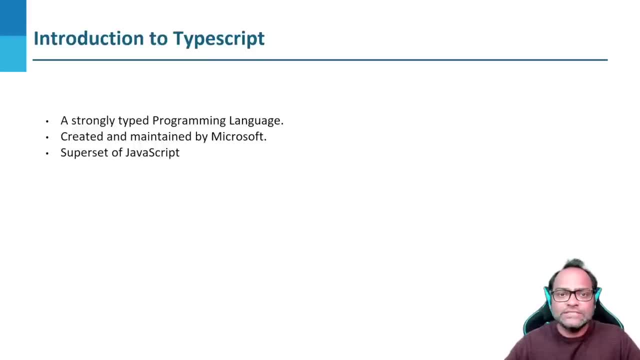 a variable, you say, okay, it is integer, it is a string. it means you are already defining or you're telling the program that, okay, this is the data type of this particular variable and it should only hold the value of that particular data type. that's what types, if it is, and it is created and 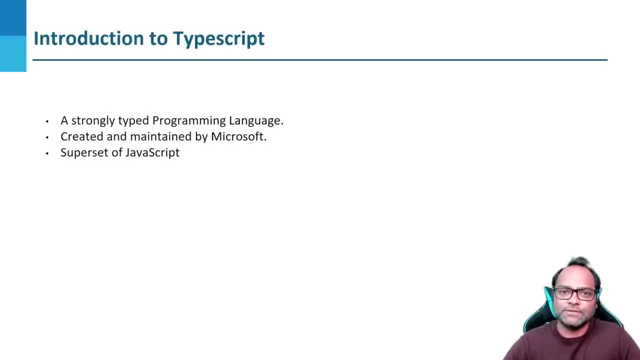 maintained by microsoft. so initially you can see that it is created and maintained by microsoft. so initially you can see that it is created and maintained by microsoft. so initially you can see a lot of people, a lot of new developers, thought that it is created by google, which was totally 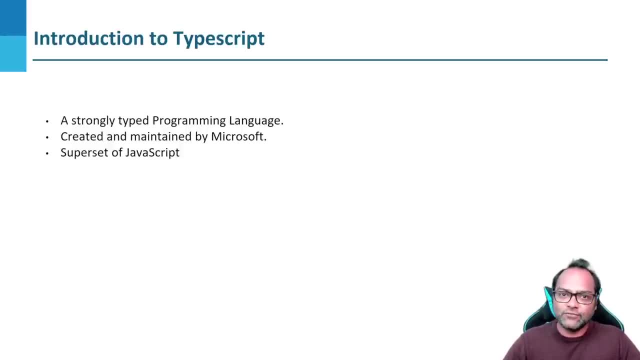 which is wrong, of course, because uh, as angular, was the first to adopt typescript. that that's why people think about uh or thought about that it is created by google, but it is not so. it is created by microsoft back in 2011 and i think around 11, uh, around 12, there was some. 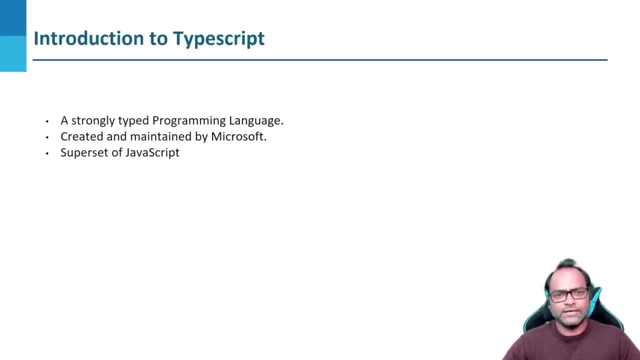 public release, which was which was available, but it didn't got so much recognition. because it was not so much recognition, because it was not so much recognition until unless google team decided that they will be writing their new framework, which is known as angular v2.0, as we learned about in. 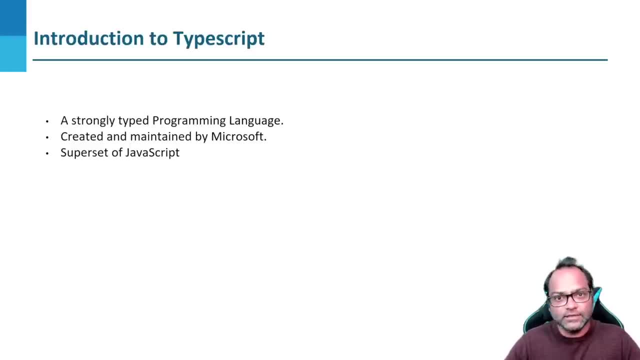 previous video that they will be rewriting the entire framework in typescript, and then people started talking about typescript and now typescript also has many versions. right now I think the version 4 is there, the major version, but I think minor version is 4.4.4. so we'll see that I mean. 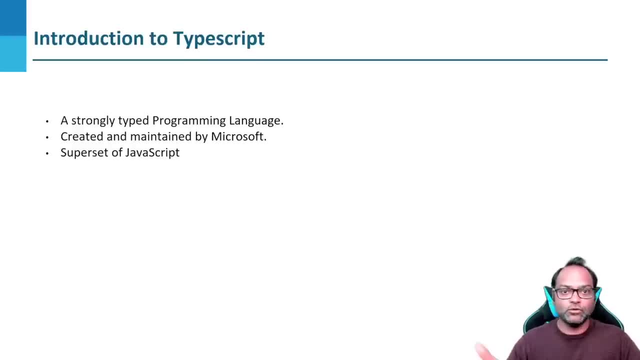 we will, of course, learn typescript before we move into, uh, angular. that's the whole idea about this particular section: that where you will learn about typescript, you will write your first program and we'll learn more about it. it's a super set of javascript, so let's. 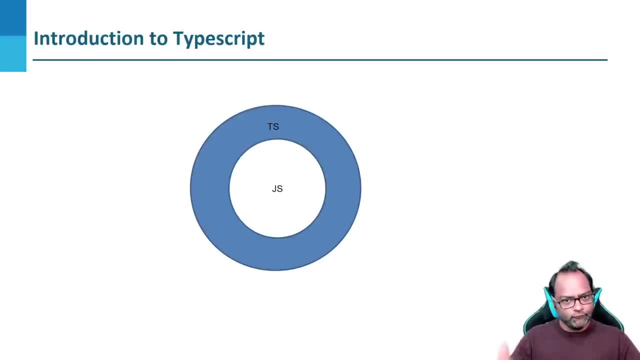 talk about this thing, uh, before, I'm sure, before coming to angular, in case you have written, uh, your front-end code, you might have used javascript and you might be wondering where is javascript and why? why should? uh? we use typescript so you don't have to worry about it. so most of the concepts which 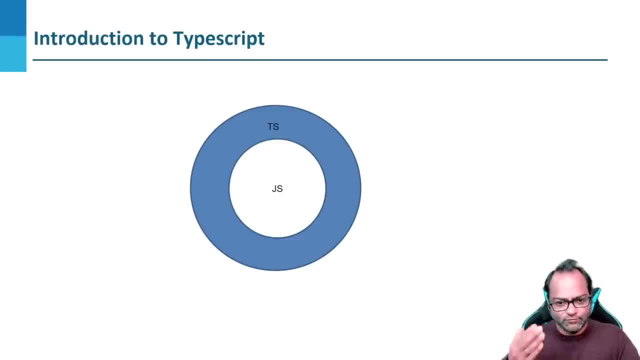 we have learned is actually same, because if you see this diagram, it says: okay, javascript is nothing, but it's a subset of typescript. so, uh, a free javascript program which you have written so far is a valid typescript program and you can actually go ahead and convert them to typescript. 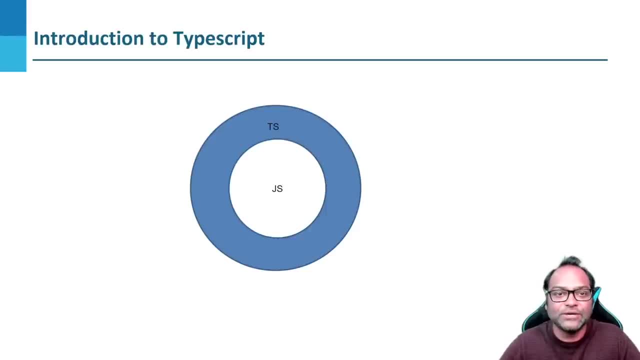 by just renaming the file. most of the cases it will work without any issue, until there's some type safety issues, that's it. but it should work. so let's see what happens. what happens by typescript, right? so why should be using typescript? so, as we mentioned, it's a superset. 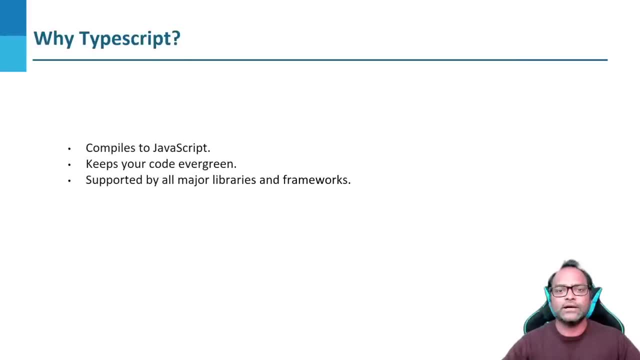 right, it's a superset of javascript. so almost, uh, learning of is very much smaller. it compiles down to javascript. now, this is. this might be something which is confusing to you. so we are saying that, okay, typescript is superset of javascript and then it compiles back to javascript. yes, that's. 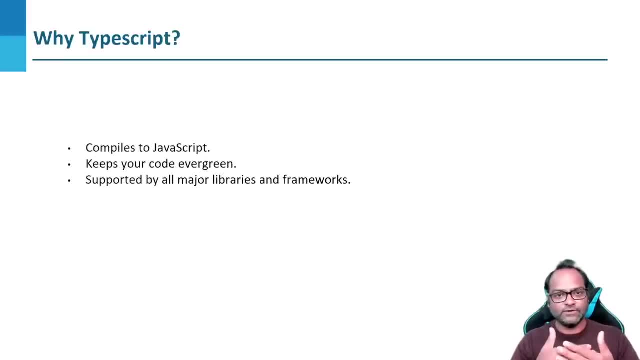 the whole idea. so typescript only provide your type safety. so once you write your program, most of the time what you see whenever you write a program or you write a code in javascript, there is no type safety. I mean, we'll talk about type safety, which will be coming up, but yeah, so the whole idea is to provide type safety to your 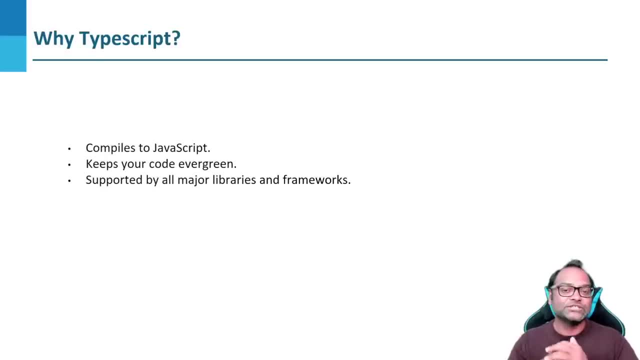 program which will be compiled down to javascript, by using which, once you actually run your program or you compile your program, you get all those errors related to type in your, in your, let's say in your- development environment, before going to protection. that's the whole idea. it keeps your 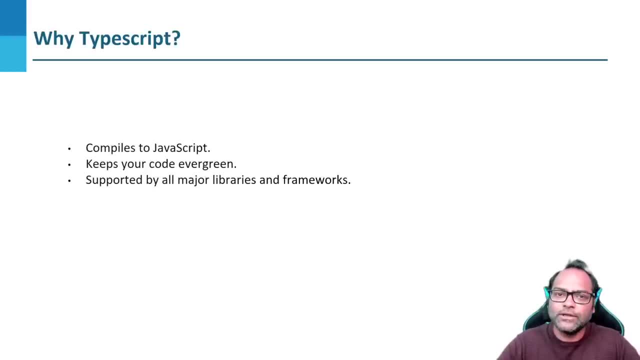 code evergreen. now, what do we mean by keeping your code evergreen? there are many version of javascript. in case you are not aware, the es5 was there for a long time. es5 is supported by most of the browser, even including i11 and older browsers. now, with latest browsers, we have es6 or es3d15, but that that's not. 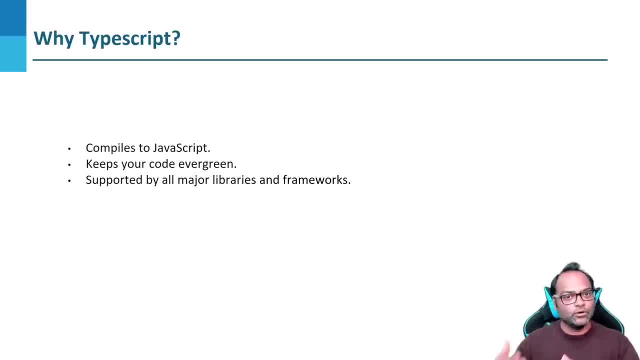 it right. so the uh, the thing is, it's going on, the, the development is going on, the features are being implemented. tc39 is the committee which uh finalizes all the features which will be added into javascript and all the browsers implemented. so es, uh, 2015 years, 2016, 17, 18, 19, 20 and then you. 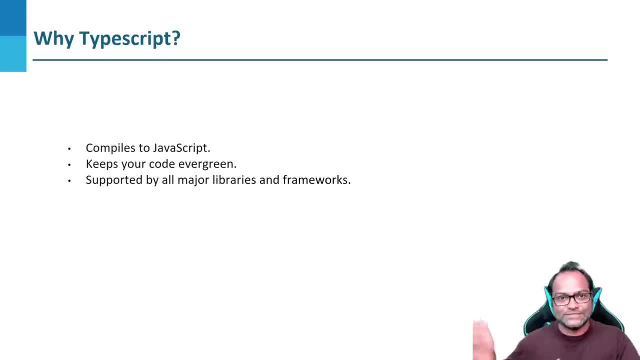 will find 21, 20 and then next those are the versions, so that it's named by year, and then next is, of course, all those experimental features. but in case I want to, I have written a code which now, as of now, uh, works with es2015. 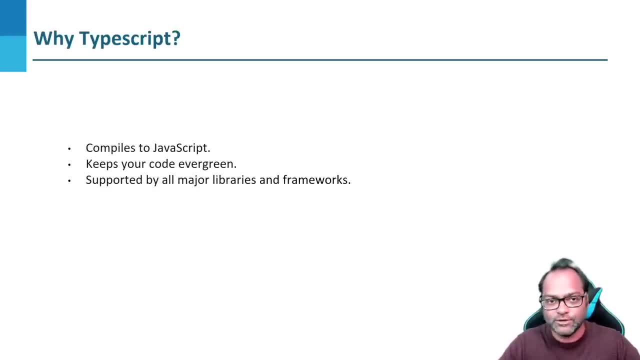 browser support. most of the browser support. yes, 2015, nowadays, all the modern browsers, now, let's say all the browsers- started supporting is 2016.. if I have written a code using es, using javascript, what I have to do is I have to actually go ahead and adopt to the new features, right, or? 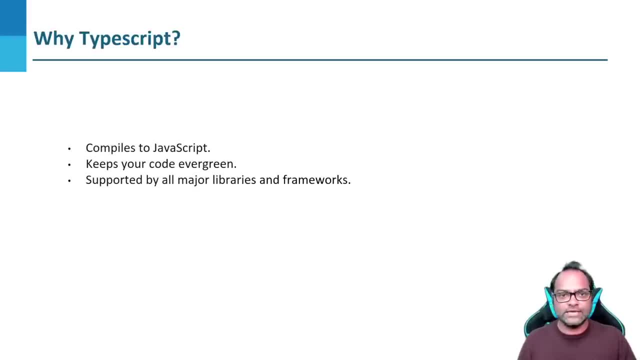 new syntax, but using typescript. you don't have to. you can just say, okay, compile down this javascript or compile this javascript to es2016, and then you are done. that's it. that's what I mean by keeping the screen. it is supported by all the major framework and libraries, all the javascript code. 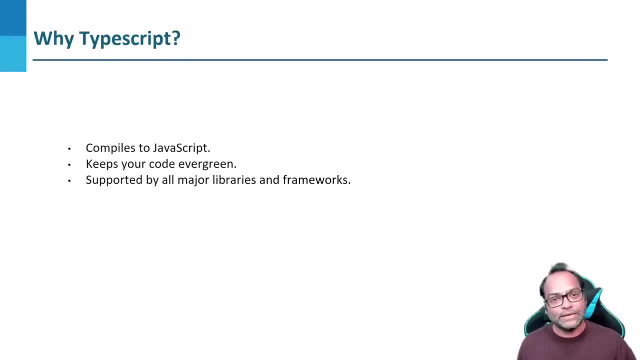 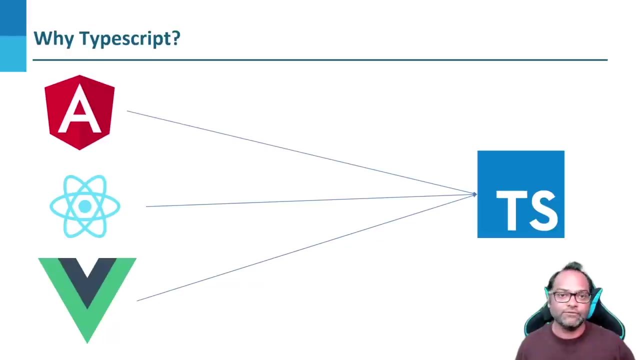 or all the javascript libraries you which you will find on npm. they do have something called types if they are not written in typescript, or most of them are actually written by script written in typescript. so of course, here you can see: react loves typescript. react is one framework. 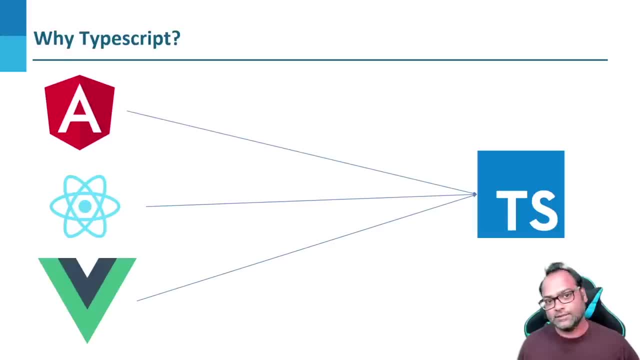 which is also one library which is not written in typescript. they use something called flow and but you can write your code. so now a lot of react developers are adopting typescript and writing their code in typescript. angular written in typescript. who the new version, which is v3? 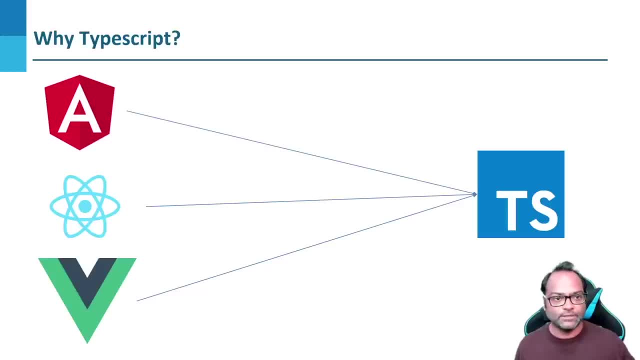 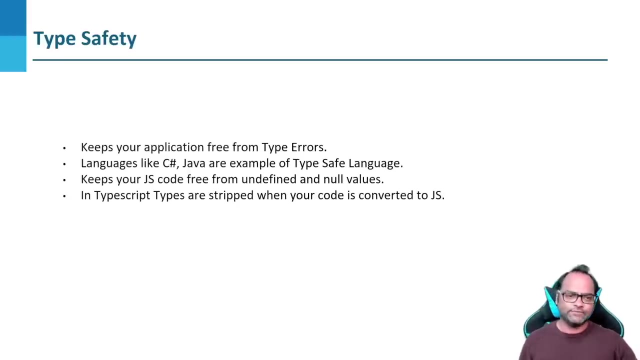 actually is rewritten in typescript. so yep, all the major frameworks, supports. even you can write your back-end code using typescript. so express js, you have nest js and all all those frameworks can be written in typescript. coming back, type safety. so what is type safety? 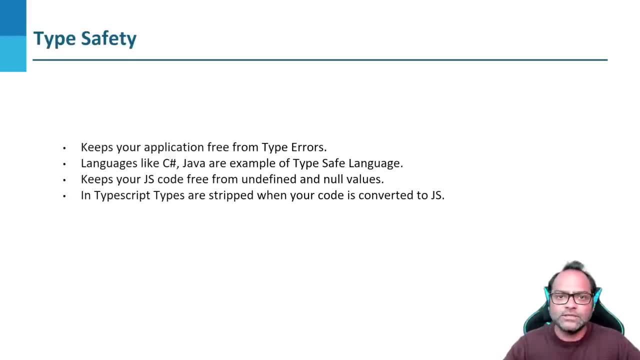 in case you have written your javascript code in past, you might be familiar with one error which we get a lot undefined, cannot find or cannot read something, or fun defined or probably null errors. why that happens? because there is no types right, i mean we, you don't. 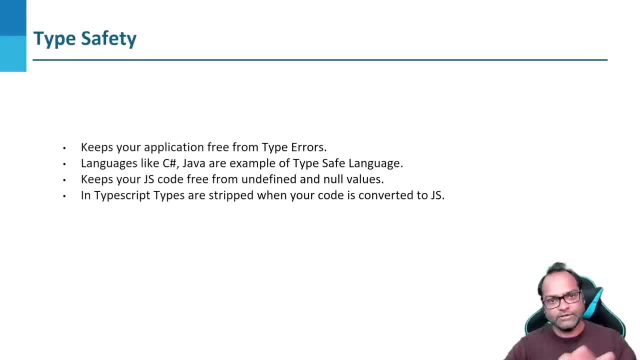 define that. okay, this particular variable be integer and it will have a default value of something, let's say zero, or it's a string, and default value will be, let's say, blank. you don't do that. you don't do that in javascript. and when we don't do that, do that and we write: try to compile our code in our browser and we try to access those. 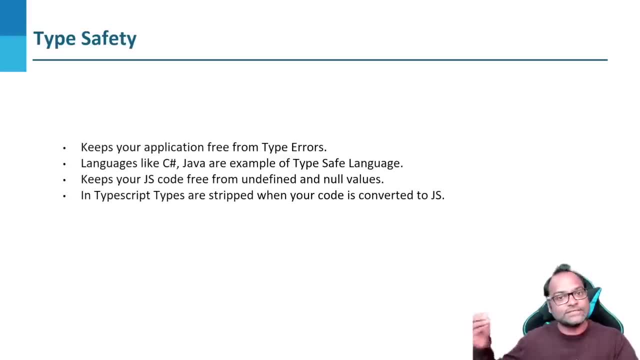 properties. or let's say, access those variables. and we try to access the properties of that variable. what will happen? in case there is nothing, no value is defined or no value is assigned or there is no data type, of course you will get an error. but in case i can get those error, the 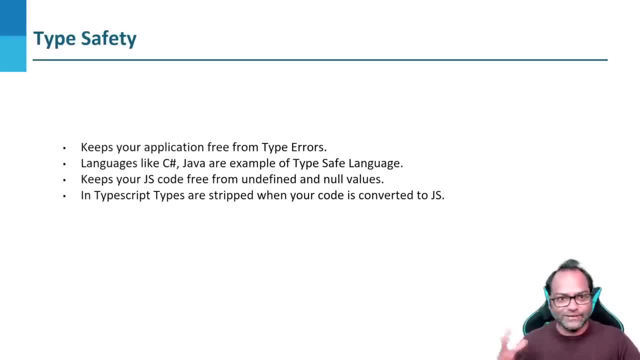 undefined and null, the most widely introduced error or most widely seen error in your javascript code while compiling your code. what i mean by compiling your code? nowadays you have lot of compilers, which is available. type typescript also comes with its own compiler, so it's known as tsc. so what we can? 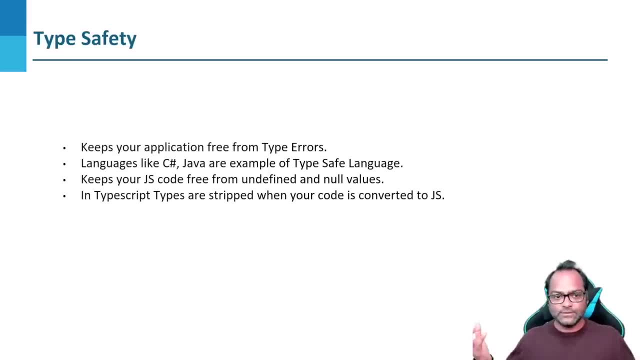 do is we can capture those errors during compilation time. that's that's what type safety does for you. languages like c, sharp and java. they have been doing from a long time. but now typescript is trying to solve that problem while writing your front-end code, or, as i said, you can also use it. 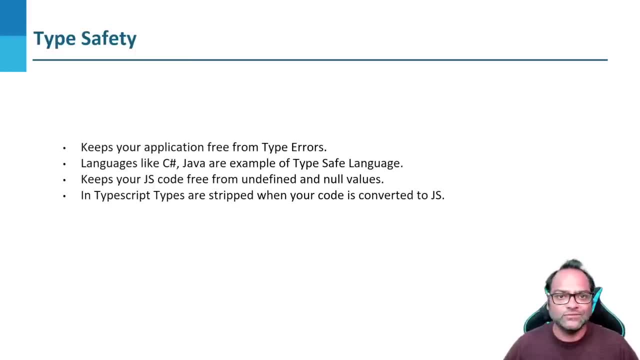 for your backend, because, of course, thanks to nodejs, you can run your javascript code anywhere. browsers you can run on your os, windows, local machines. right, it's just one thing. but one thing now. as we said, type script will be compiled down to javascript. you cannot run typescript code directly into the browser. that's not possible. 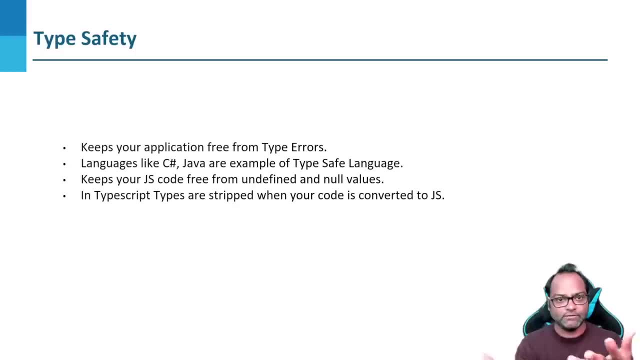 typescript code is something which is just for your purpose, for development purpose- and it will give you the output of javascript code right. so once you get javascript code, you can go ahead and execute your browser. your browsers cannot understand typescript. there is a new runtime environment called dino. 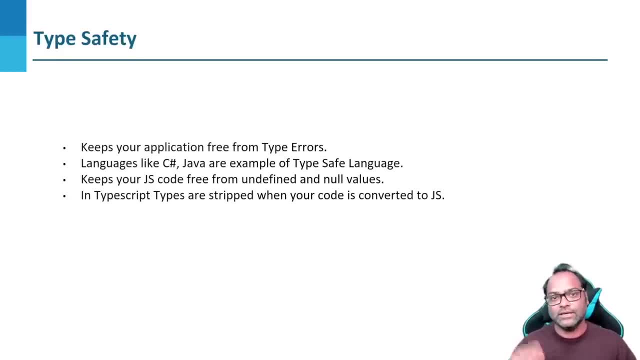 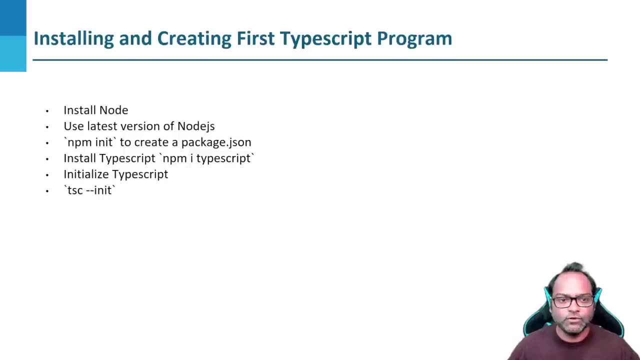 DENO TypeScript. you can write your TypeScript code and you don't have to actually compile it down to JavaScript, It will just run. We will see some code where we will talk about type safety, But before that, let's go ahead and create our first program and see how we can run. 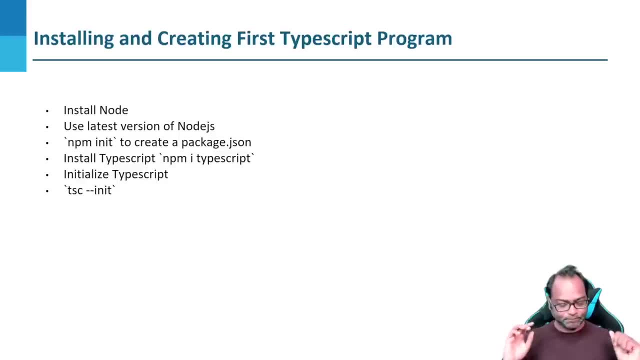 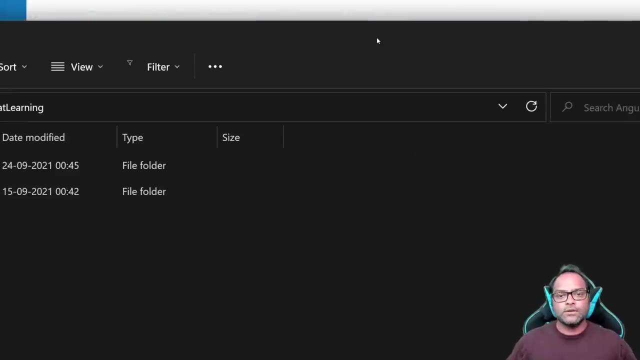 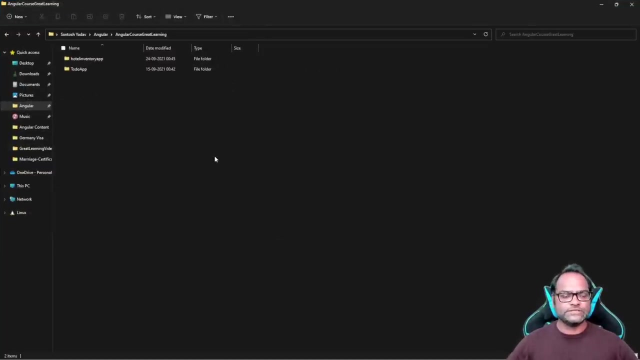 create and compile our first TypeScript code back to JavaScript code. So what I'm going to do is I'm going to create a new folder which we- which I will name it as TypeScript demo, And we will keep the entire code which is related to TypeScript in this particular folder. 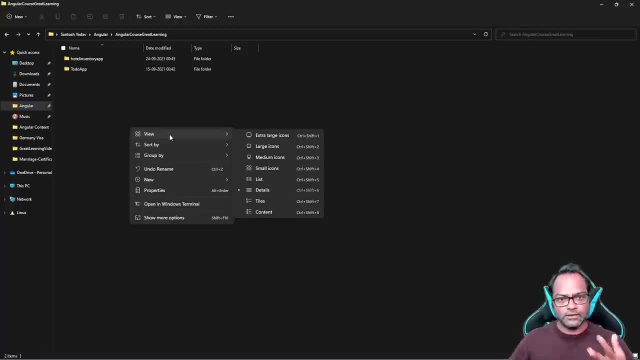 And this code will be shared with you. So you can either just follow the video or follow the code, write the code by yourself, or you can download the code and play around it. That's up to you how you prefer. So let's create a new folder. 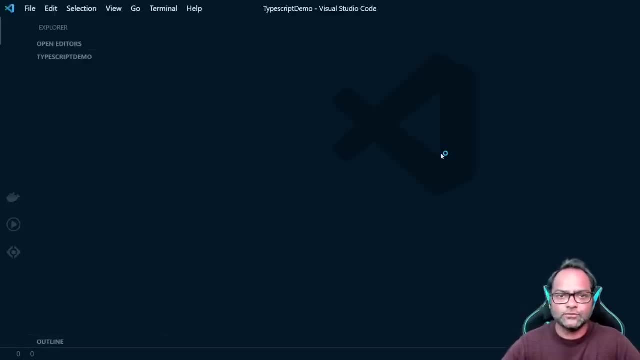 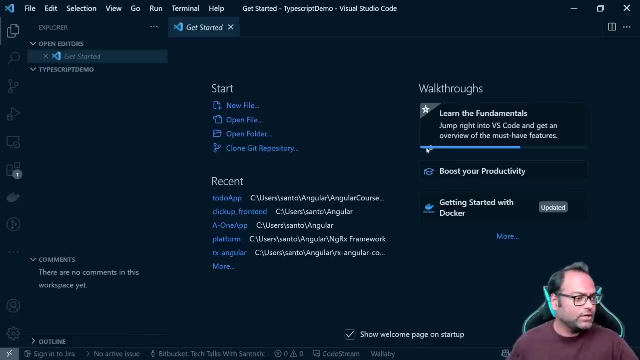 So I'm using VS code as my editor. You can use whatever you want to, but preferred VS code. I think it. I mean it is available for all the all the OS. Let me show you the link from where you can download it. 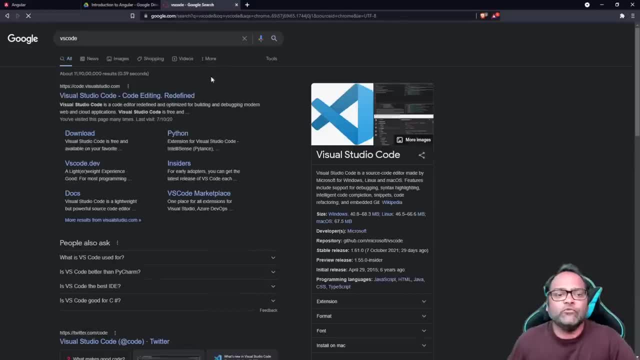 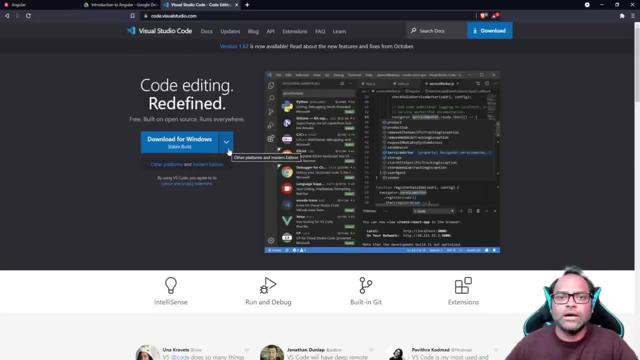 So you can just go to Google and type VS code and codevisualstudiocom. You can go ahead and download the latest version, which is available right now. I'm using windows and it gets automatically updated, So I don't have to download it again. but in case you are using other browsers, just 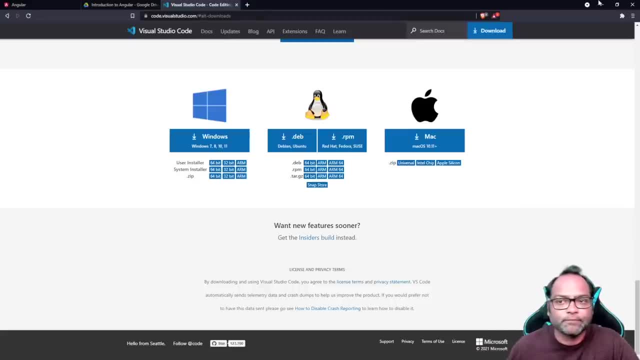 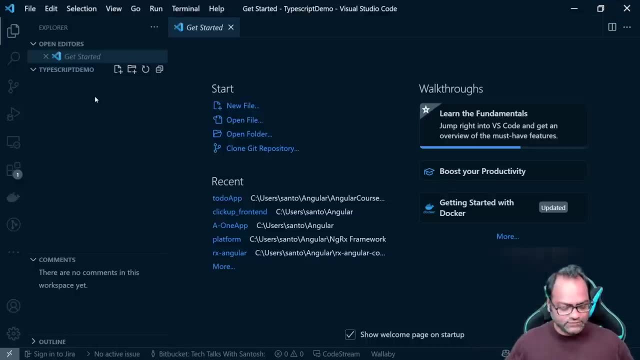 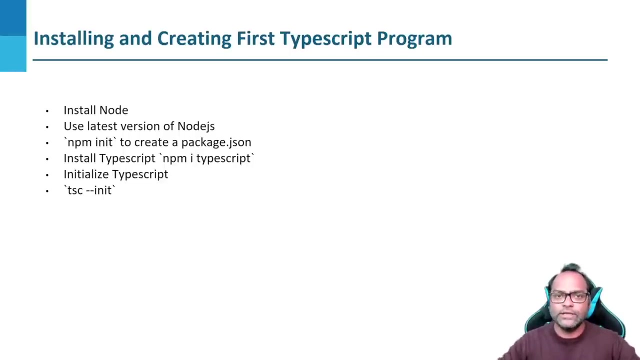 go to other platforms and install it. So now Folder, or our workspace, is available. So let's follow the steps to create our first program. So what we need is, uh, we first need to install node. node is required. In case you have already installed node, just go ahead and verify the version. 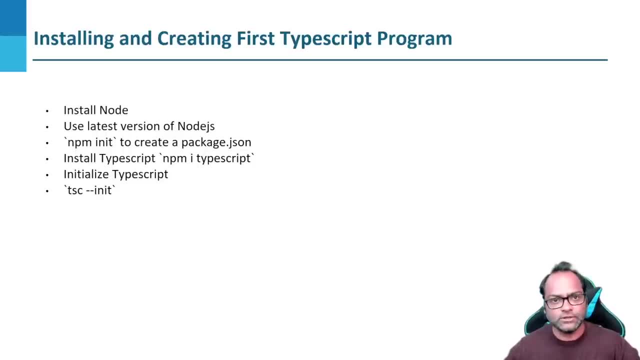 We are going to use a node above 14 because that's what is supported by the angular latest version. angular 12 and 13 also supports node 16.. But, as I said, I'm not going to use node uh, sorry. angular 13 as of now. 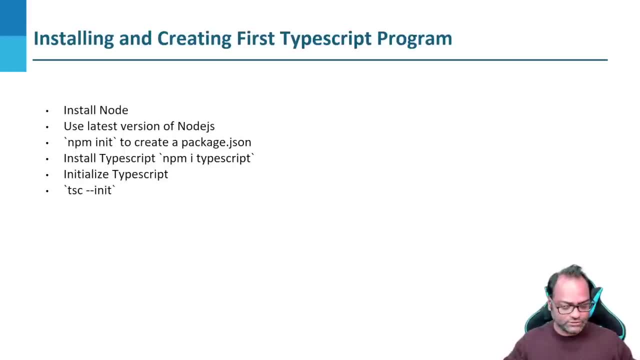 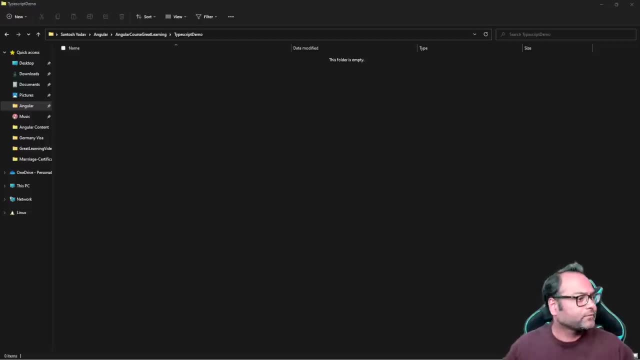 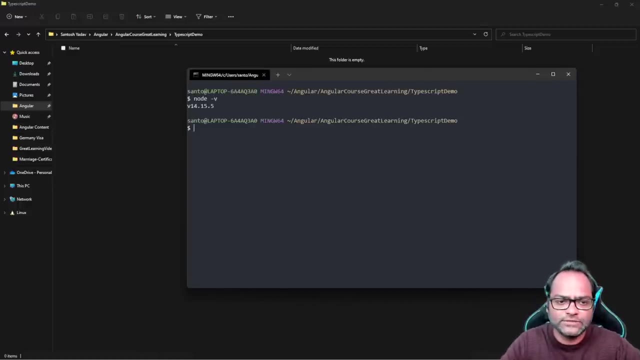 Uh. so let's install or just first check the version. So I'll use windows terminal to verify the version which you have installed. You can just say: node, I can be, it will give you the latest version. My latest version is 14.15.5,, which is okay, because I want to use uh, angular 12 and 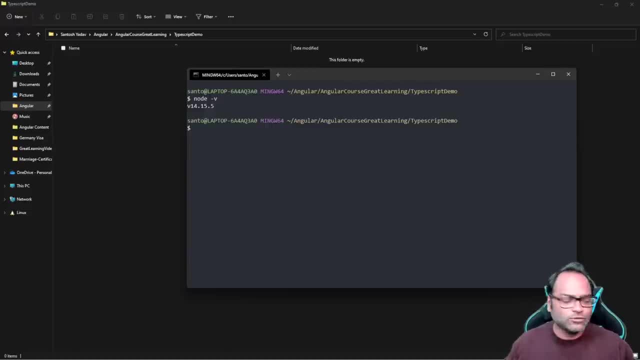 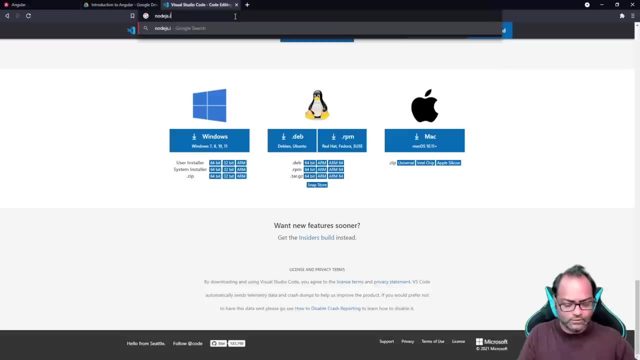 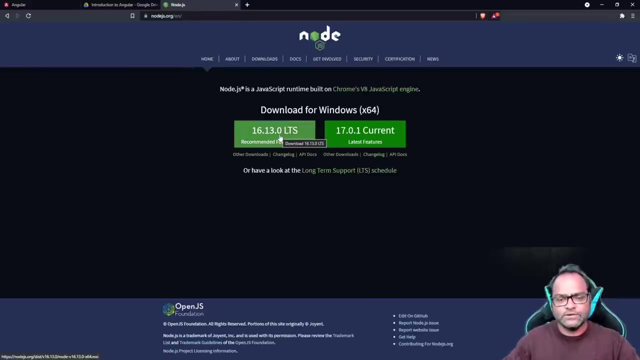 it supports it. Okay, In case you don't have node installed, doing it for the first time, So you can go to nodejsorg And, uh, you can see. latest stable version is 16.13, as I said, and you can download it. 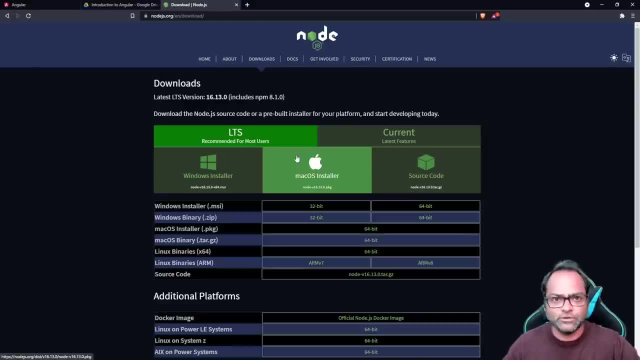 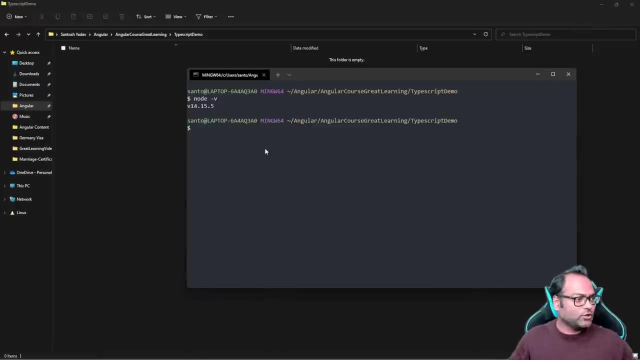 as per your OS. By default, it is giving me windows option because I'm using windows, But in case you have Mac OS or Linux, it will probably prompt you with that particular setup. Okay, So once, uh, you have installed node, let's see what we have to do. 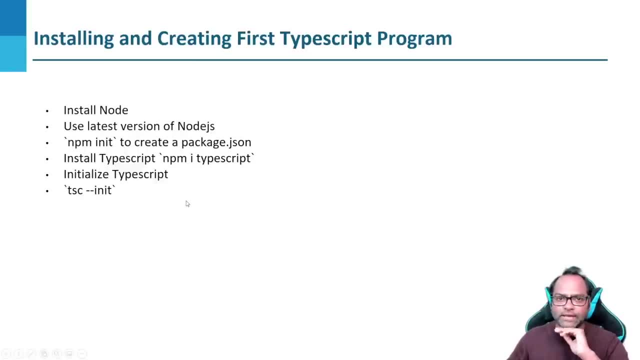 So you uh need to do npm init to create a packagejson file- Uh, we will talk about a little bit about packagejson file later. and then we have to install TypeScript and then we need some, uh, we need to initialize TypeScript. 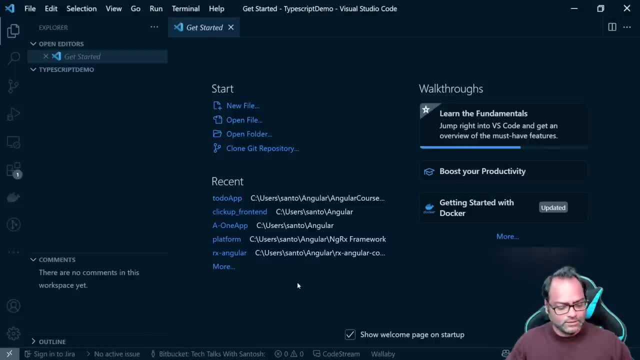 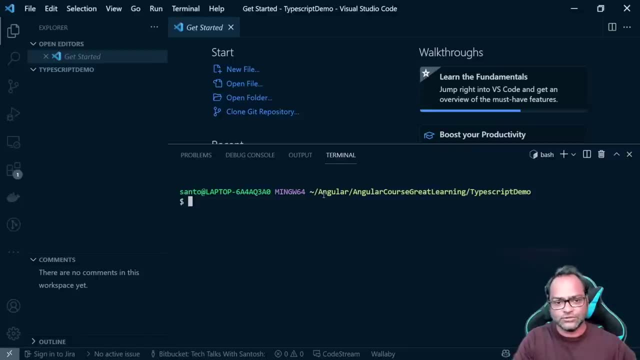 So let's talk about the steps. So this is my terminal, And uh, now, first thing which we wanted to is we wanted to create a packagejson file, So which is npm init. This is the command and it will ask you a few questions. 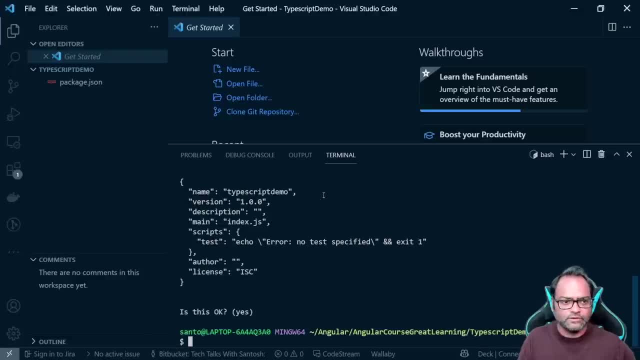 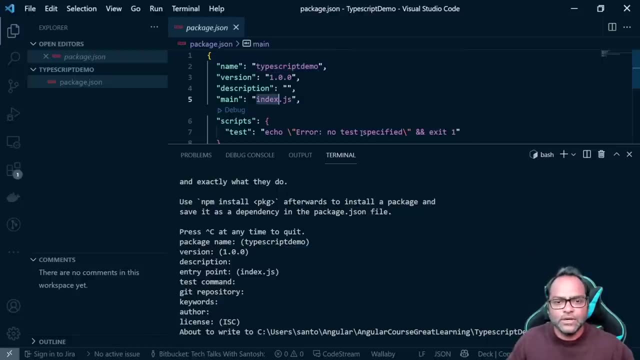 You can just press enter and move on. We just wanted a few things which is like name and version. That's it. And main indexjs is fine. So this: once we have this packagejson file, now we need to install TypeScript. 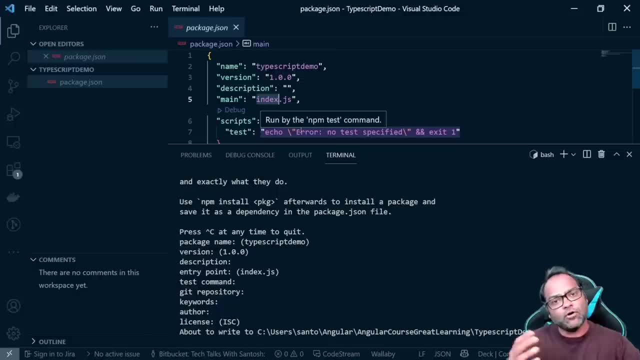 So this packagejson file will keep track of all the packages which you use And which is installed in your uh workspace. So that's why we we are going to use this packagejson. This packagejson is really important file because once you publish your code on npm- 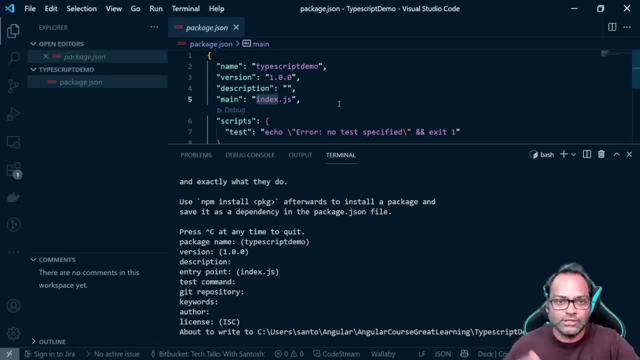 uh. npm actually uses all the information from this particular file. What are the packages you depend upon? What is your name, What is the name of that package, What is the version of that package? So everything is actually taken from here. So now we have our uh file. 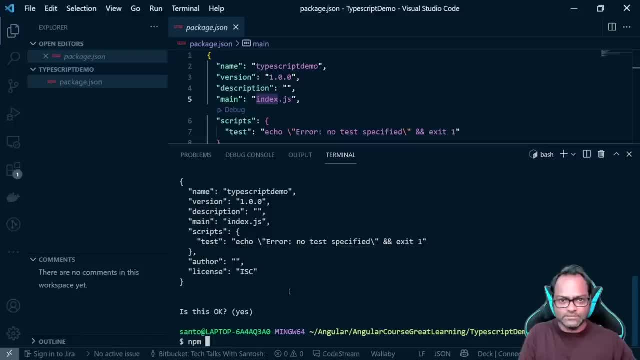 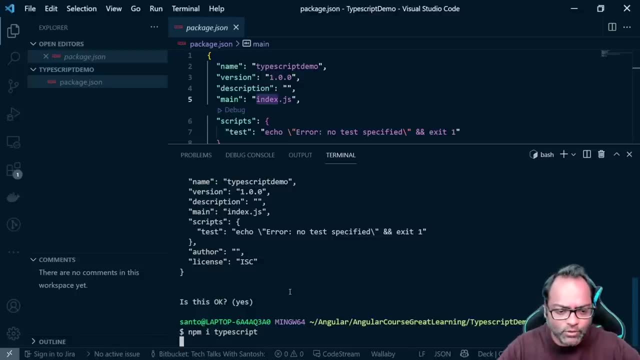 We have our packagejson file Now, install TypeScript. So I'm going to install TypeScript. I'm going to run this command: npm, install TypeScript, and it will probably give us- probably let's see- 4.4.4.. Yes. 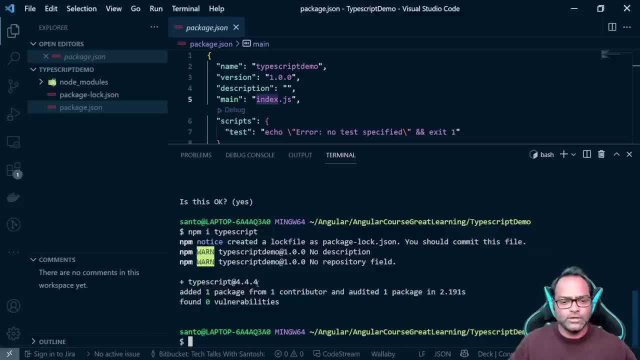 As I said, that's the exact version which is available right now, And now it gives you a node-modules folder. This is where all the packages which you installed will be kept, Nothing which you should check in. So this is only for your development purpose. 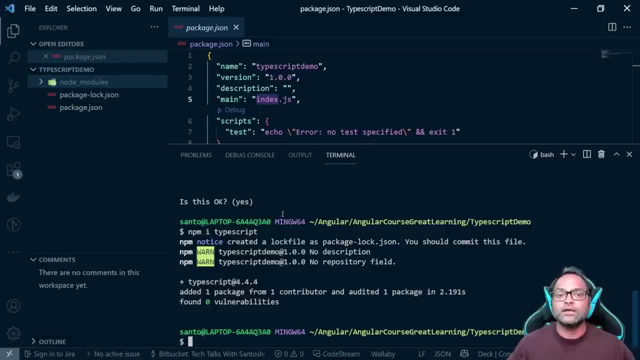 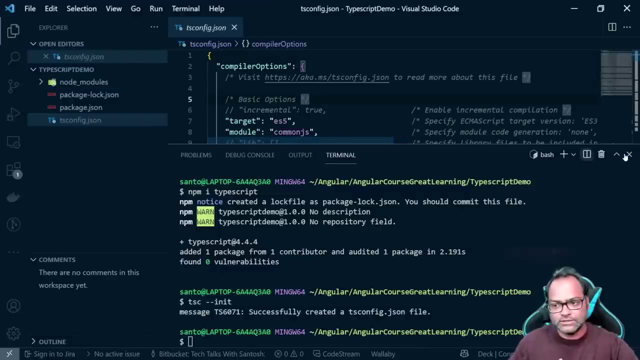 Now we have our TypeScript installed, We have our packagejson file. We need TypeScript configuration file. So we need to run tsc-get, So we have to do tsc-init, hyphen, hyphen, init, And you will get a file called tsconfigjson- really important file. 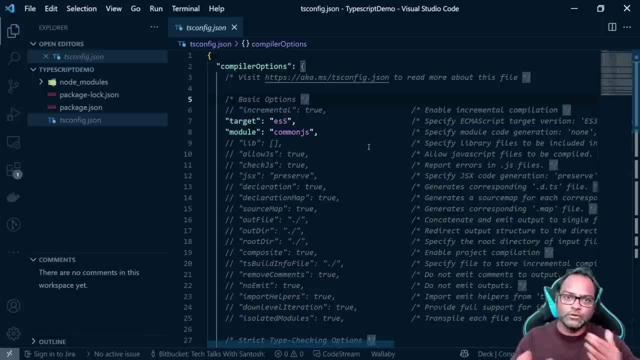 This is the configuration file which, remember, I spoke about. you need to change a version and then you can compile your JavaScript to ES 2016 and 2015.. That's the file. So this is where all the magic happens, right? 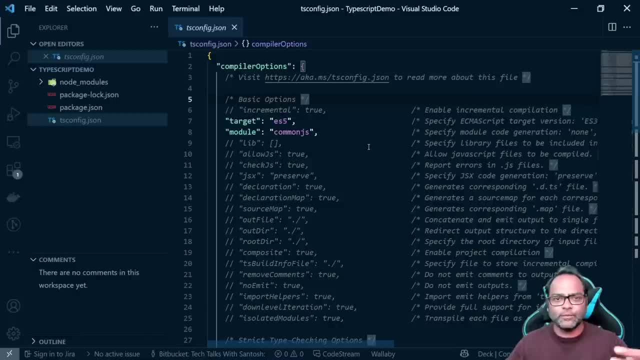 So right now we are going to just stop. Let's talk about the first two properties, which is target and module. So target, by default, is ES5.. ES5 is, as I said, the JavaScript version which is supported by all the browsers. 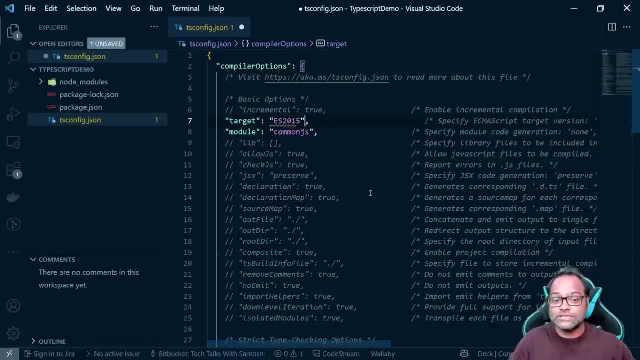 All the modern browsers, though, they support ES 2015,, so I'm going to change it to ES 2015.. Module is something which is for where you want to actually run your code, whether you want to run it on browser, whether you want to run it on your OS or your command prompt. 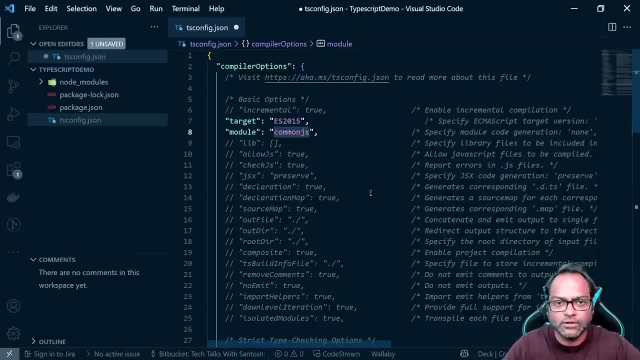 or from your machine- local machine, Sorry, not local machine, but yeah, on your OS, not on browser. So CommonJS, we are not going to. we will let it be CommonJS right now In Angular. you will see it will use ES next, which is of course for browsers. 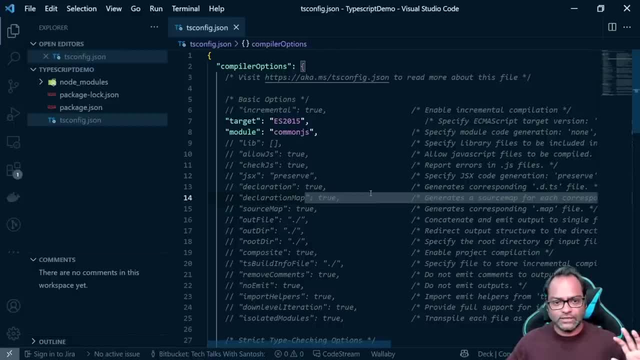 So that's it. So I changed my target to ES 2015 and module just kept it CommonJS. There are a few more properties which we will discuss about later on. Now let's write our first file. So I'm going to create: 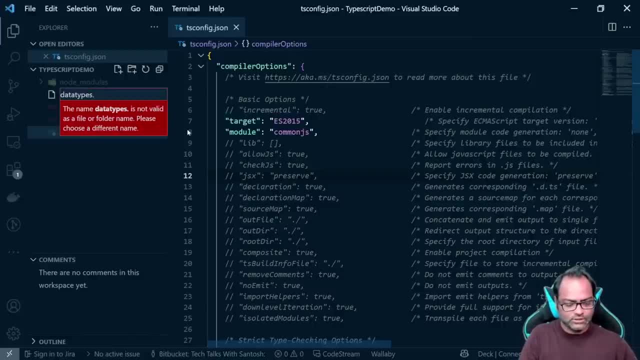 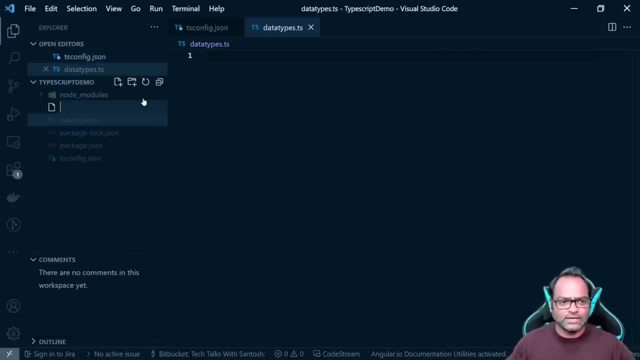 A file. I'll name it as datatypests, So all the TypeScript files will have extensionts. But before we do that, let's create a JS file and see what's the problem. I mean why there is no type safety. 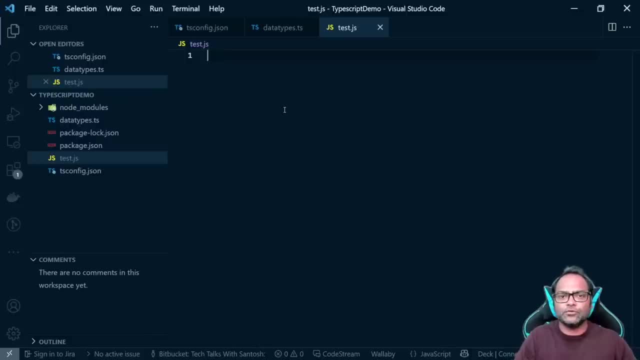 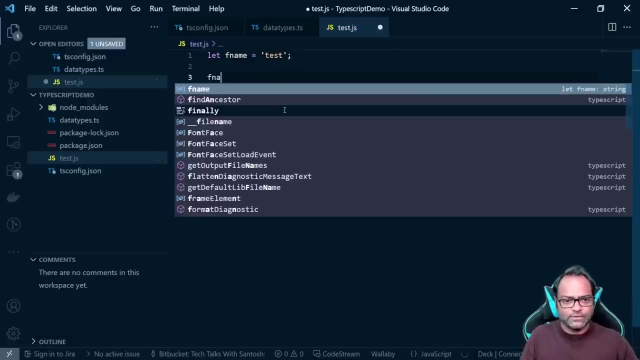 So in JavaScript, whenever you declare a variable, what do you do? So you do. let let's say, I want to create a variable called fname, and probably you will be saying, okay, this is test, right, But JavaScript also allows this. 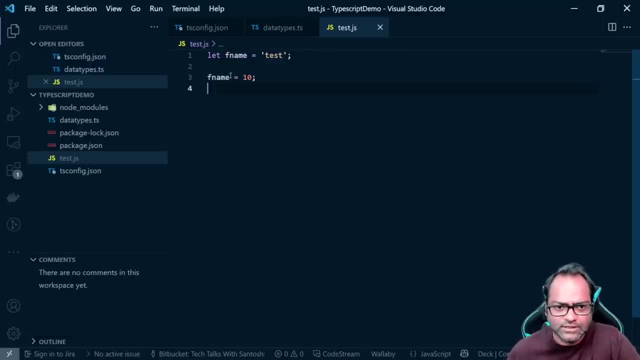 So you can see, actually I declared a variable called fname and then assigned a value, a number. It works, It doesn't give you any issues, but it causes a lot of issues once we have hundreds of lines of code, and now we lost the track. 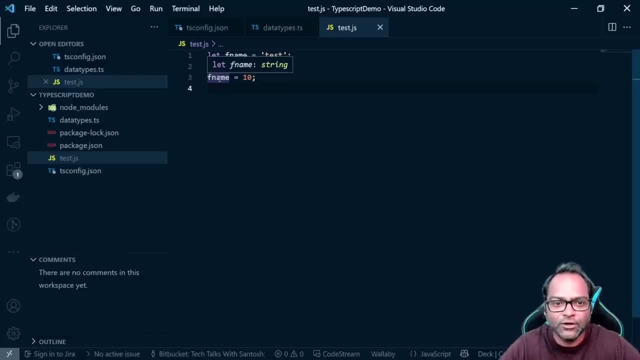 Okay, What was the variable type? And then we tried to read, Or let's say, Let's say, use some function which is actually for a string, but the value is number. What will happen? Of course, it will give you some error. 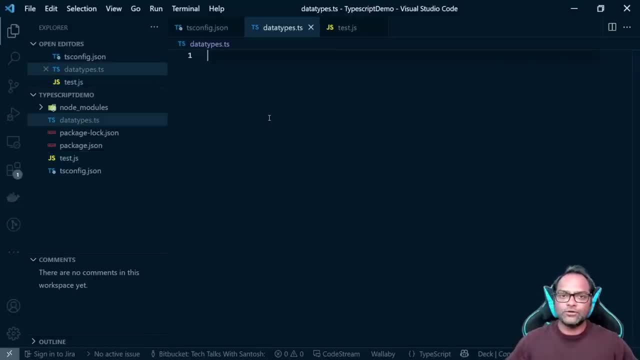 That's what the problem is. Now let's go to TypeScript. So I'll create a variable, I'll call it as a name, and let's say it is shawn, which is not last name but name, And now try to give it as a numeric value. 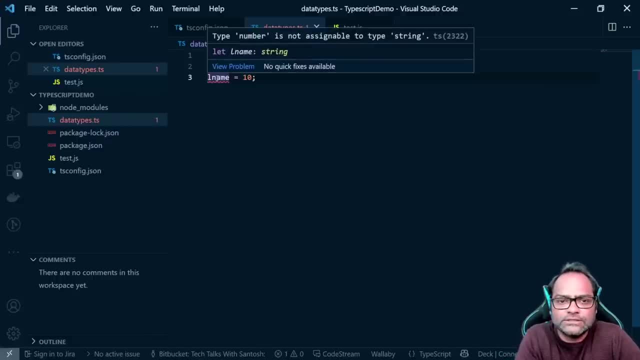 So in TypeScript it will give you an error. It will say: okay, this type number is not as unable to type string. because of course I mean: this is: uh. you, while initializing the variable, you said: okay, this is string. 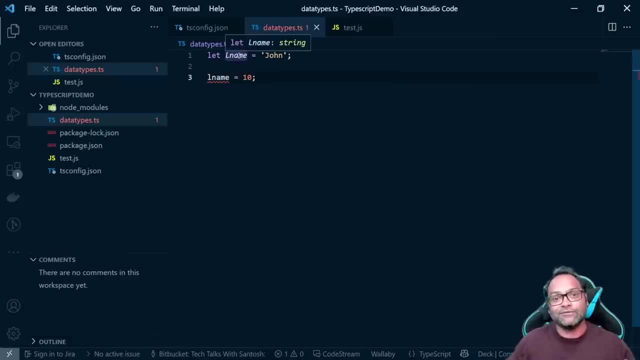 And how this is happening. We will talk about it. I mean, we are not, uh, if you see, we are not giving any data, but somehow it is saying, saying okay, this type of string. So we'll talk about that as well. but yeah, this is just to introduce you that okay. 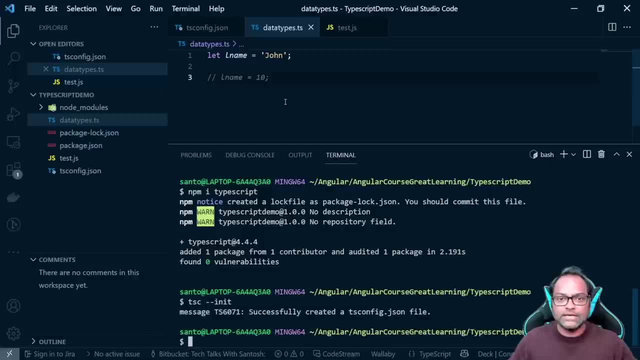 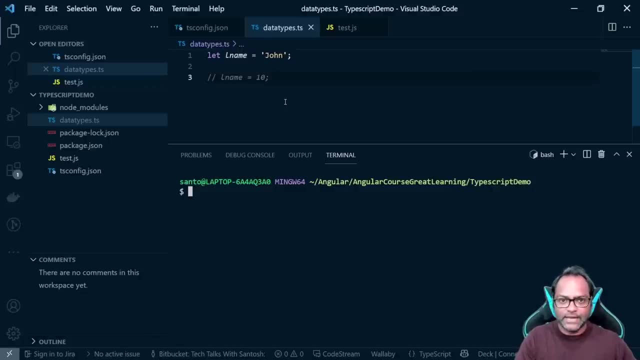 this is what type safety is. I'll comment this out and see how to compile this code. So here, uh, what we will do is uh, TypeScript comes with its own compiler called TSC, TSC. Now, once you do TSC, it will compile down this code to JavaScript code. 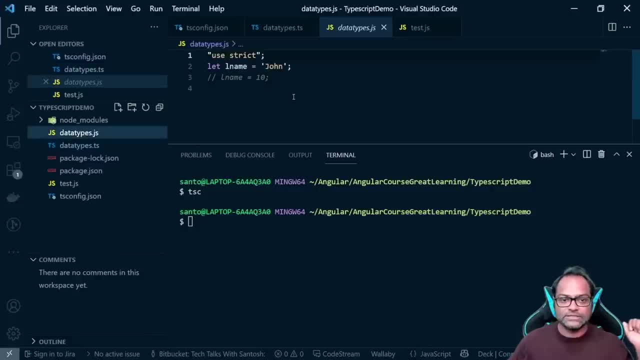 So it will create another file with same name. So you can see its name: uh, datatypesjs, and almost it contains the same code, but I mean it's a JS file. So this, this is the output which is generated, but we will be doing few more things with 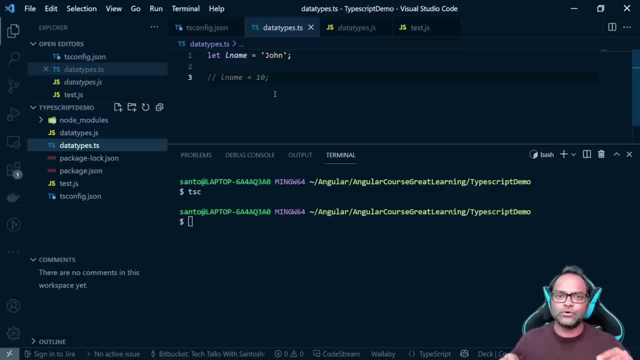 our this datatypejs file. This code was just introduced. It will introduce you how you can compile your code and how you can write your TypeScript code and how you can get the ES 25, ES 25, 15 version as your output, or JavaScript version. 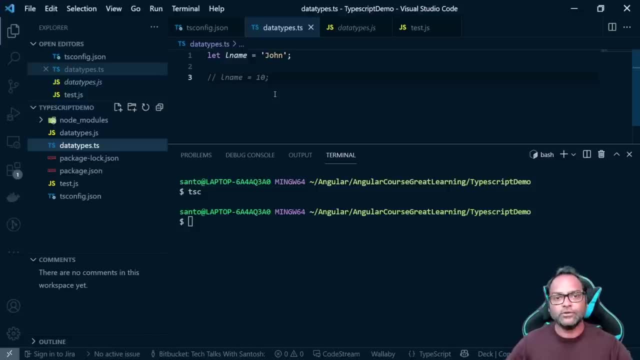 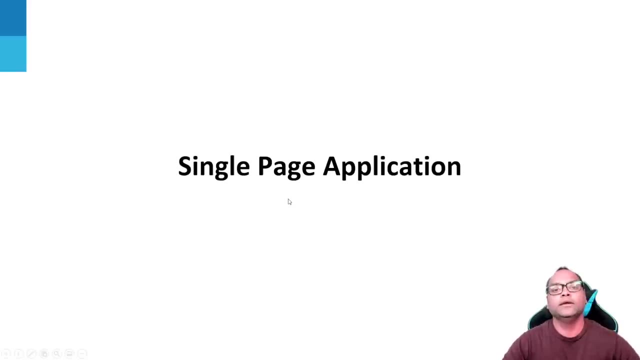 as your output. So that's it from this video. I'm we'll move on to the next video now. In this video we are going to talk about single page applications. I'm sure, in case you are, uh, going through some job requirement or you are going through 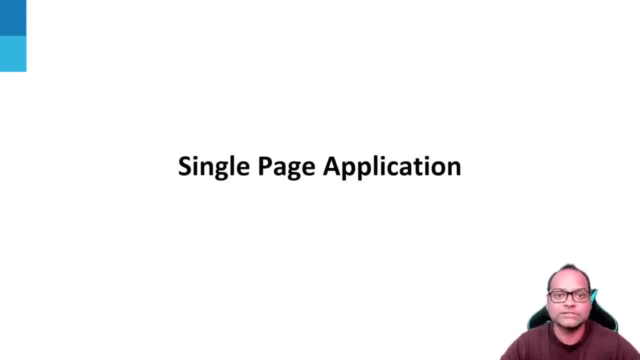 some uh uh, development, uh, using new frameworks. they all support single page applications, right, So it's it's one of the widely used uh word nowadays in technology. So every framework, all the major framework which we have, they support SPA. 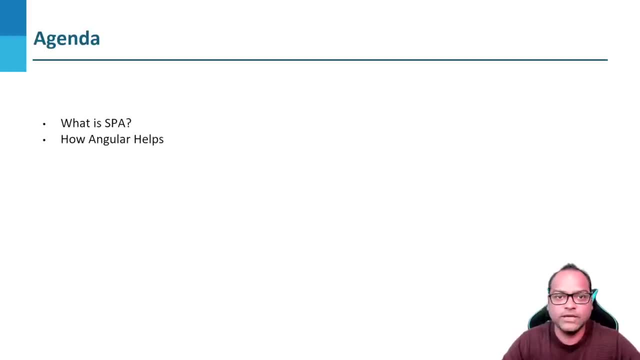 So let's see what we are going to do in this video. So we will be talking about what is SPA and we'll also talk about how Angular actually helps you to build single page applications. So, as I mentioned, SPA stands for single page application and all the modern frameworks. 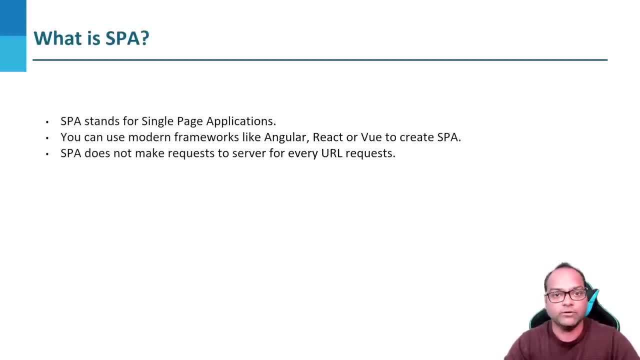 Angular JavaScript- Uh, you are also Angular Java and react and Vuejs- all those frameworks supports creating single page applications. So what's the difference? So in older days, whenever we used to create a webpage, we used to create multiple pages. 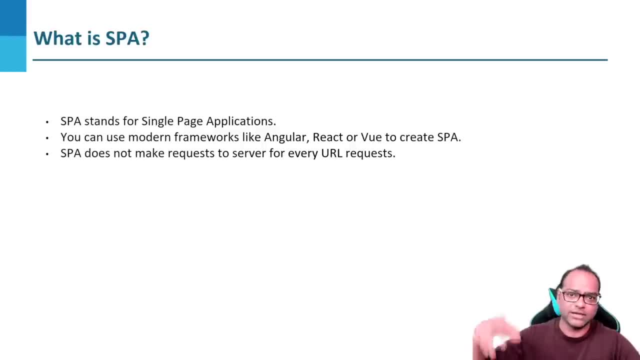 for each and every view. The problem is, of course, we are actually, uh, rewriting most of the estimates we cannot reuse. And um, another thing was whenever we used to switch between The URLs. for example, let's say, you have page called about this, you have page about 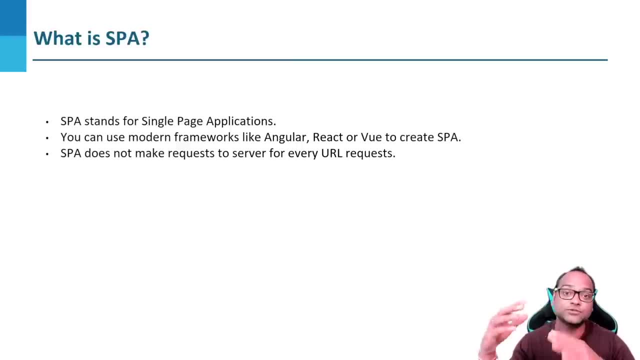 a home or homepage. So what? what used to happen is there used to be a page refresh. The reason was, whenever you click on a URL, the entire compilation of that code used to happen on server side. So it's like- I'll give an example of ASPX pages which were like: uh, which will uh. 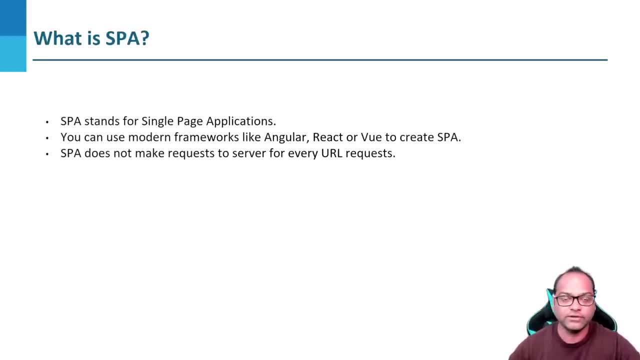 which were used long back And it was created by NET framework or using NET framework. So we used to create ASPX pages where, like uh, for each URL, we will be creating each page And whenever you click on a page, it request goes to server. server will identify okay. 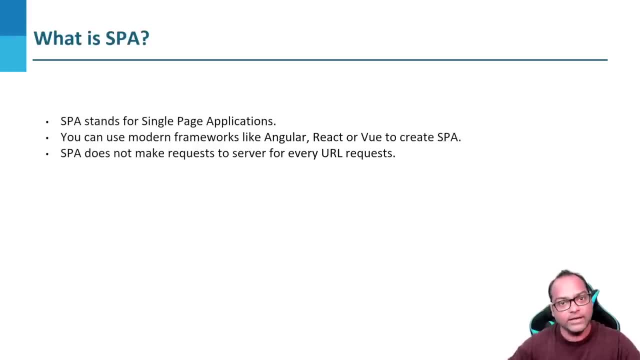 this is the page which is which is requested, And then it will compile down all the pages and then it will give you the estimate. Then a lot of developers thought, okay, I think this is not the most efficient way. What we can do is we can just give the static pages as it is, rather than actually compiling. 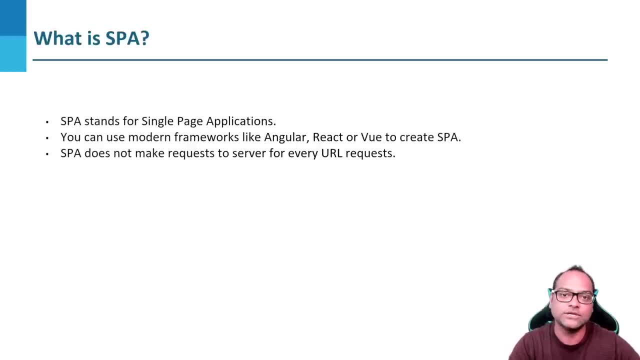 everything on server. We can actually send all the resources to the client browser and then it can render it, No compilation needed. So that's where, that's how, SPA came into picture. So in SPA what will happen is all the resources actually to render everything will be sent. 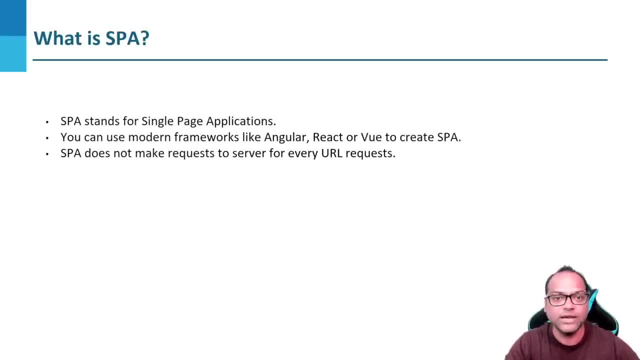 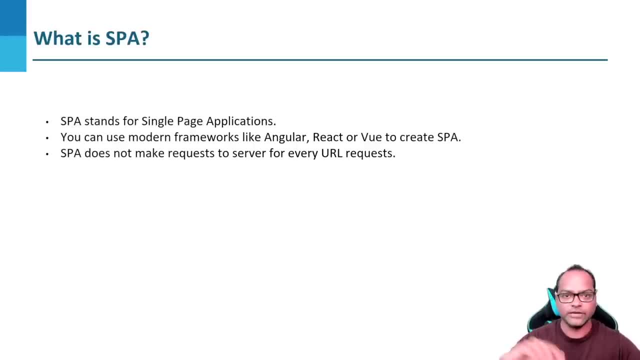 uh to uh to uh to get the data from there. it will be a request, but it will not reload the entire page. That's the difference in SPA, Even though I have multiple URLs. in frameworks like React, Angular or Vue it will be like. 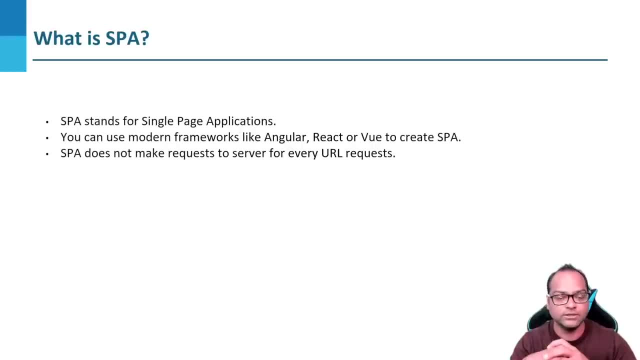 a bunch of JavaScript code which will be required to re-render something. So, in case, let's say, I have FOM, I have about us and I click on about us. So some JavaScript code which is already, which will be, uh, rather either download. 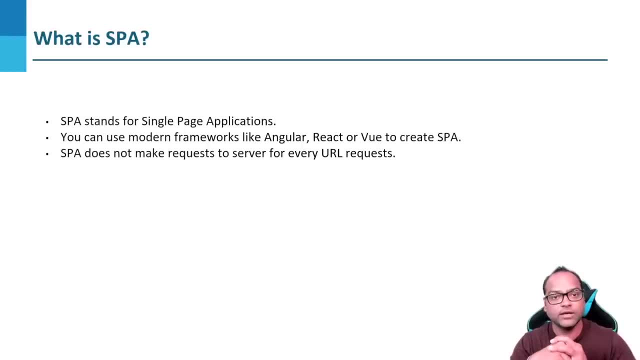 downloaded or which is already present, will just go ahead and change that particular view, so it will render whatever information is required on that particular view. so that's that's how spa works, how angular helps. so angular has its own routing engine. so whenever you click on some urls, angular 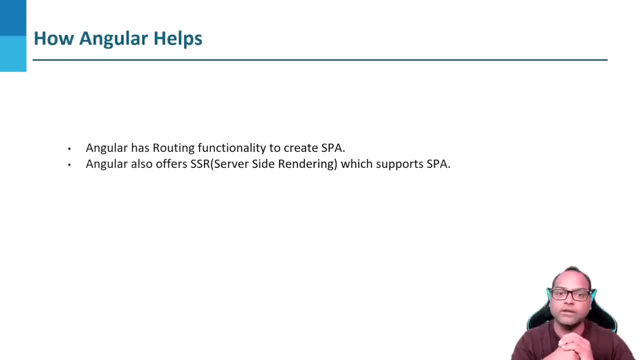 knows which view to render, and that's how it happens. angular has its own library called angular slash router, which we will learn about and see how it how you can actually do everything. you can request for a url, you can create your multiple urls- friendly urls, i would say- or html5. 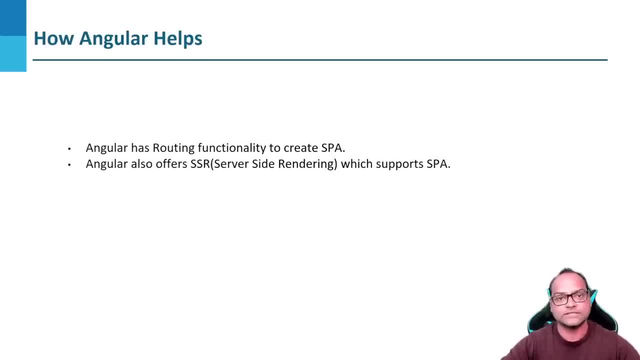 urls now which is used, and then angular also offers ssr server-side rendering. yes, it's available, but again, it's not like the older days where the request goes to server and then there is a full reload which will never happen. so it's not the full reload which happens, but here angular will. 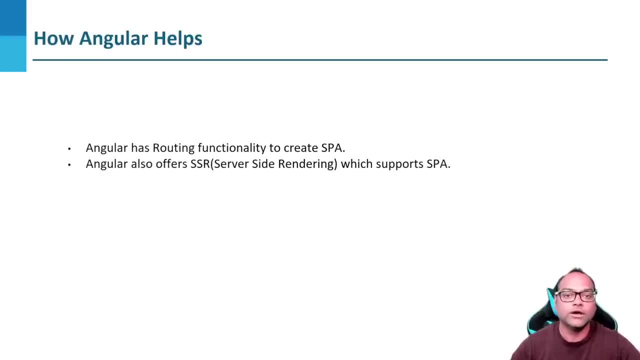 actually go to server and then compile and it will give you whatever data which is required with the entire page. so it's not like the difference between ssr and spa is ssr is good for seo, search engine optimization. in case you for you, your focus is more on seo, go for ssr or there are other tools available to. 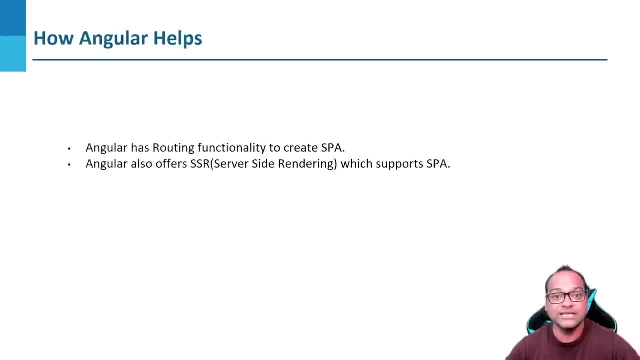 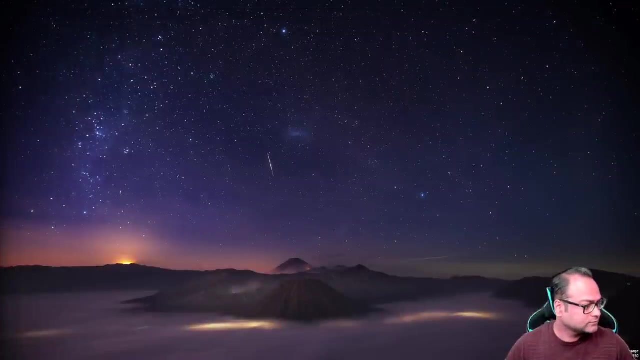 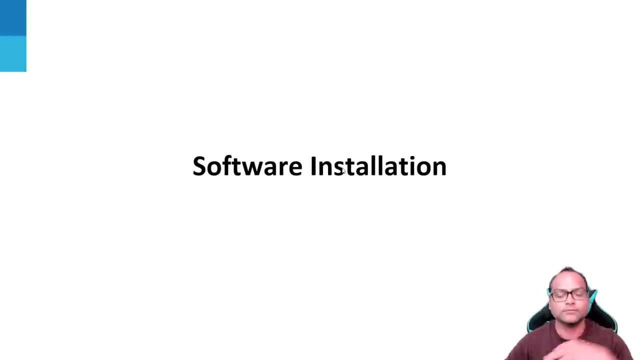 create your static pages. for example, there is something called scully, which you can also use. so this is it from spa, and now let's move on to the next topic. so before we go ahead and learn about, of course, typescript and angular, we need some softwares to 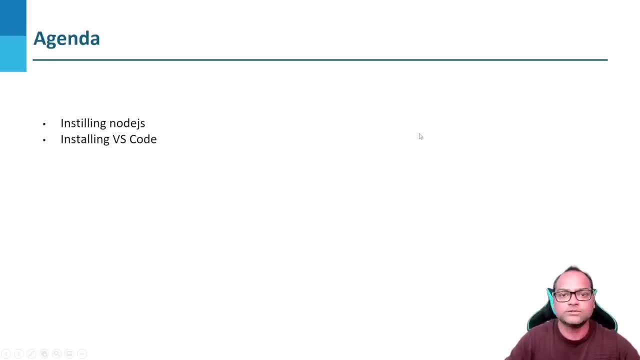 be installed. so what we are going to need is we are going to need node js and we are going to need an editor. editor is your choice. i am going to show you how you can install vs code, and i use vs code personally. so let's go ahead and. 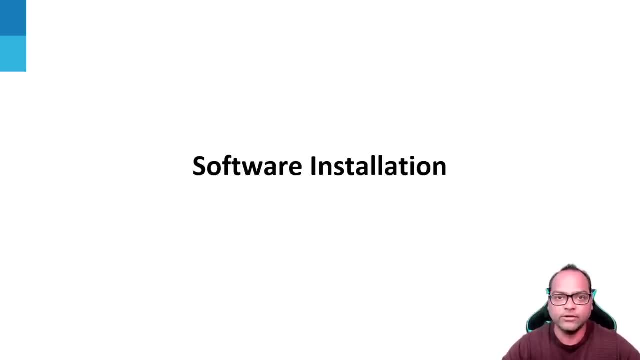 so before we go ahead and uh, start learning about typescript and angular, we are going to need some softwares to be installed, and that's what we are going to do in this particular video. we are going to need vs code and we are going to need node js as well. so, uh, editor is your choice, vs code is the editor. 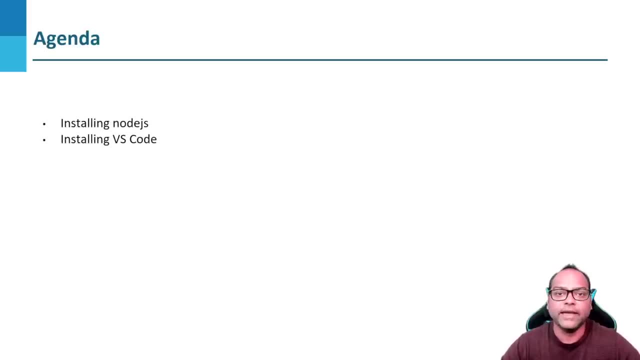 which we are going to use, but node js is mandatory and you can use any editor of your choice, apart from vs visual studio. don't use visual studio because it's like heavyweight and it has a lot of things right which we don't need generally. so what we are going to do is let's go ahead and 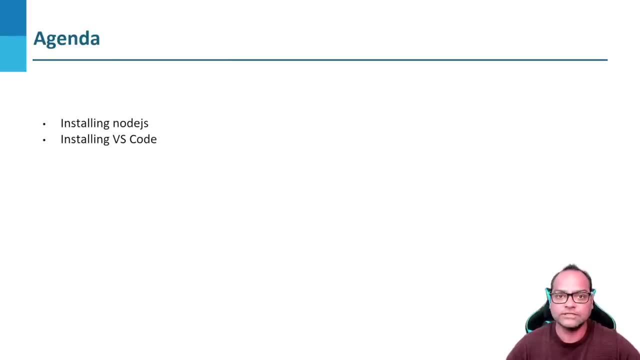 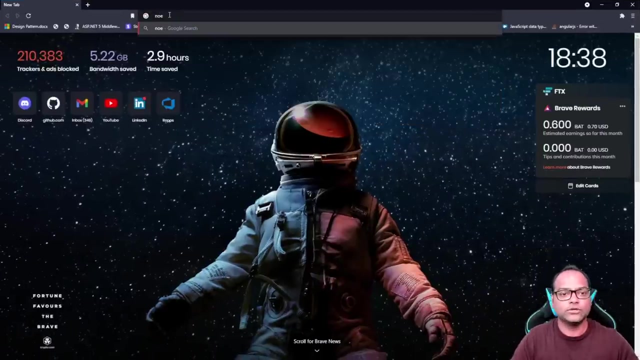 install node js and then we will see how you can use install, how you can install vs code or uh, and if you prefer any other editor, please feel free to install that particular editor. so let's go ahead and see node js. first to install node js, you have to visit this site called nodejsorg and there are 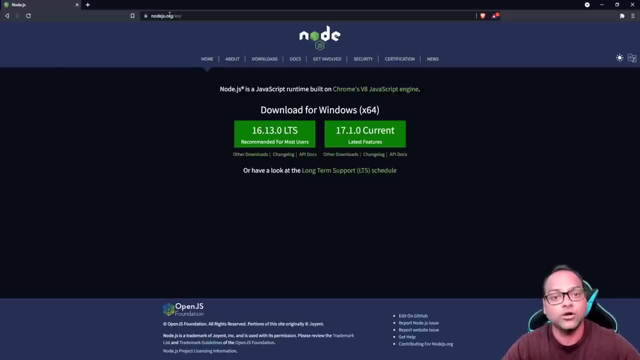 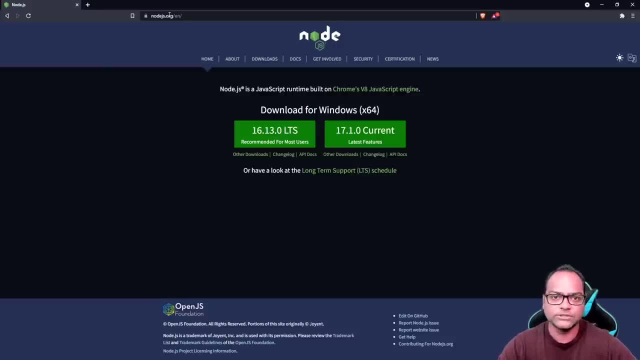 never need. so don't install current because, in case you are using it for development, there may be some breaking changes, uh, so we will go with the latest table version, uh, which is 16.13.0. so it says: okay, this is lts long term support, and let's see first how you can. 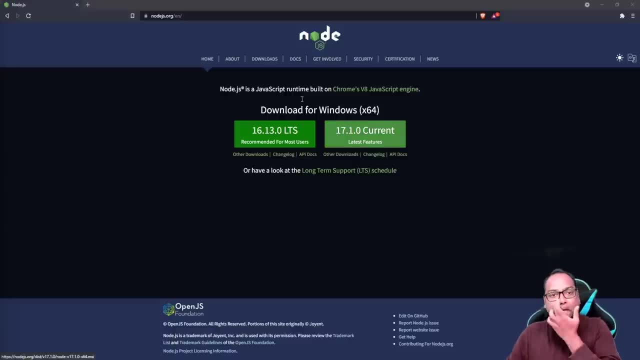 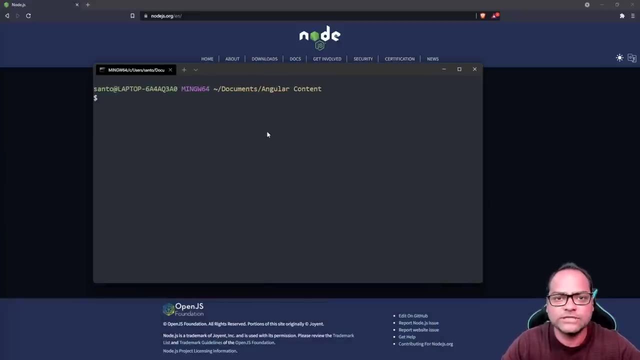 install the latest version of nodejs. so let's go ahead and install the latest version of nodejs. so let's open a command prompt and we will see how we can actually, uh, verify which version of nodejs is installed in our machine, and then we will go ahead and install the latest, latest version. 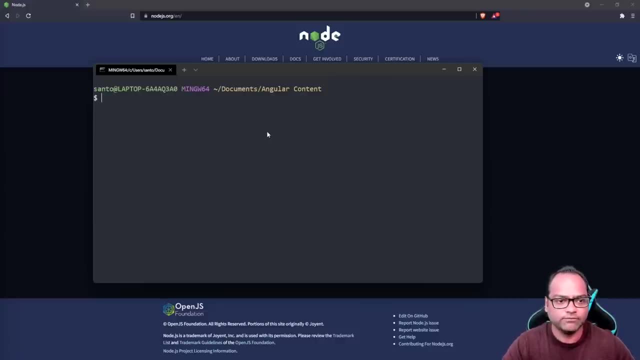 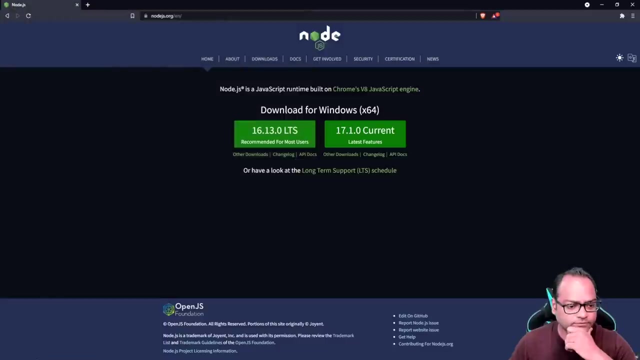 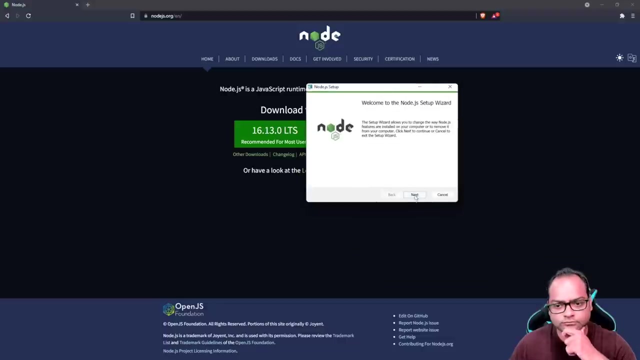 so i actually updated nodejs few days ago for my laptop, so we will see. the latest version which is available is 16.13.0, but let's go ahead and install it anyways. uh, so let's go ahead and start the wizard, and uh, right now, as i have already had, 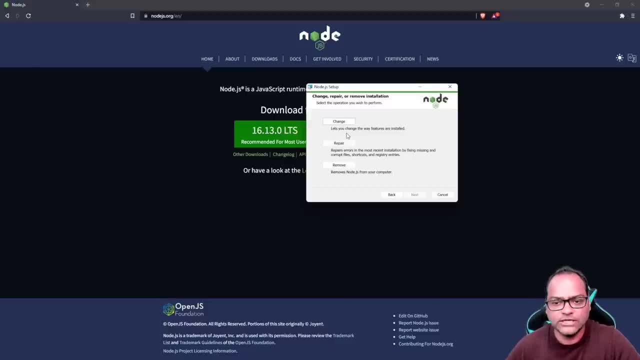 the wizard. and uh, right now, as i have already had the wizard, and uh, right now, as i have already had 16.13.0 available. it is saying: uh, do you want to change, or do you want to repair, or do you want to remove? so i'll click on change and i will change nothing. so that's, that's what we are going to do. 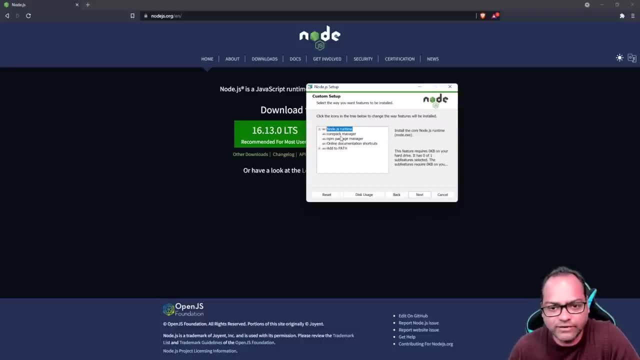 right now. so you have nodejs runtime, which is required. we need a node npm package manager- we will talk about npm in a few seconds- and of course, i need all the other features, so i'll just click on next: automatically install necessary tools. this is something which 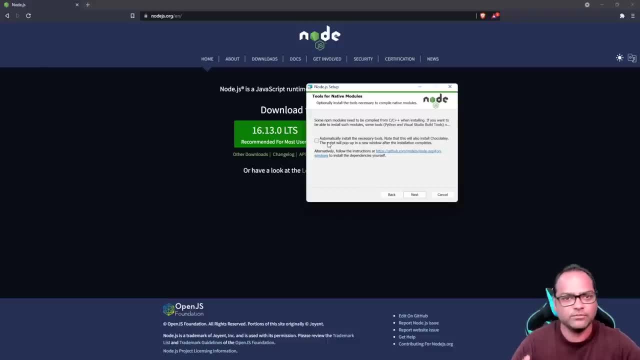 if you are probably installing it for first time, go ahead and do it, but i'm going to skip it right now. so let's go ahead and click next. and it is asking me, if okay. so it is asking me to allow to change- uh, change- on my application, which is okay. 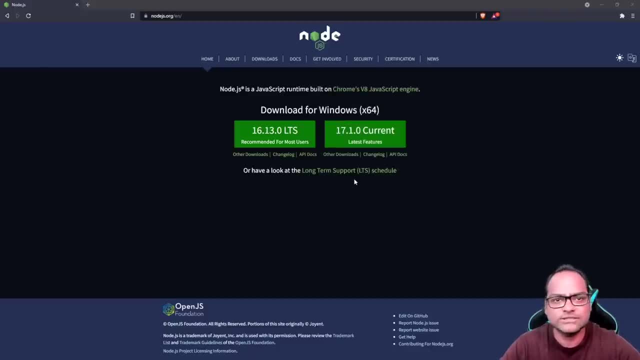 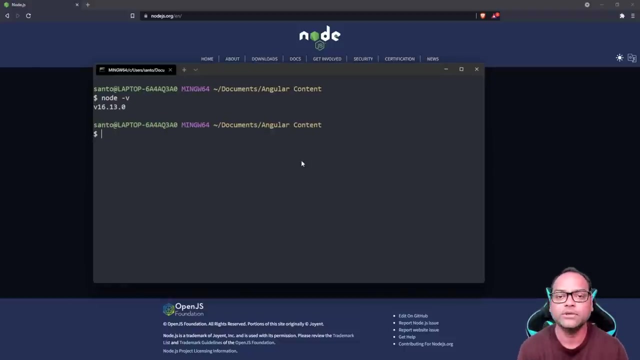 and this is it finished, right? so, in case you get some error, uh, just let us know, uh, we will try to help, or uh you may find some uh widely asked questions on stackworth in case something goes wrong. now. next thing which we need is npm. why, again, npm is a node. 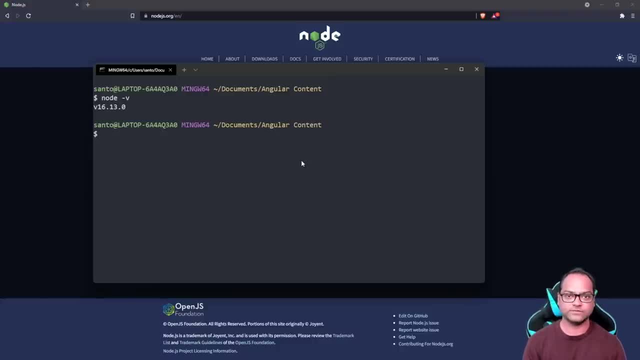 package manager which will be used to install any packages which will be required for you. so we are going to use it for to install typescript. we will also see npm being used, uh to install angular cln, and we will also see npm being used when we want to install any other packages in. 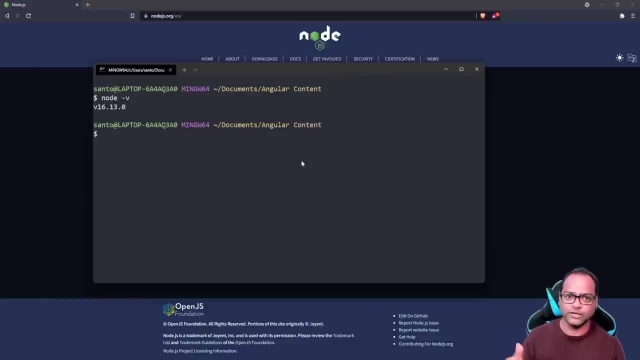 case you are coming from dotnet or java background. in dotnet you already have some. you have already called nuget, which is the package manager. in java or mobile world you have maven to install packages, so it's similar. so the only thing is: no npm comes by default with node, so you don't have. to install anything. you don't have to install it separately. earlier, in older days, nodejs and npm were two different things, but people started using so much that node just decided to make it as part of the node build itself, so you don't need to install again. there are 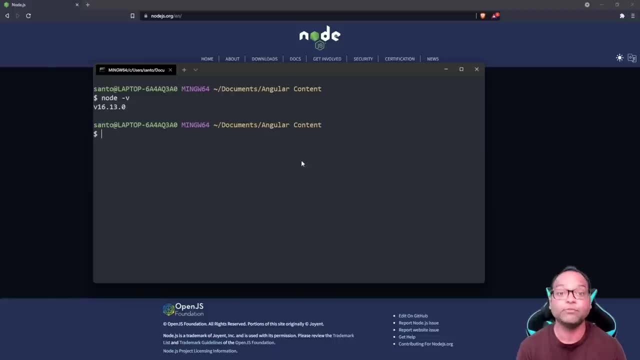 other package managers available: uh, which may you, uh, which you may use in your day-to-day work in future. so you have uh yarn and you also have pnpm. so those are two other package managers, which is which you can use. npm, as i said, is already installed, so you can see npm hyphen v. 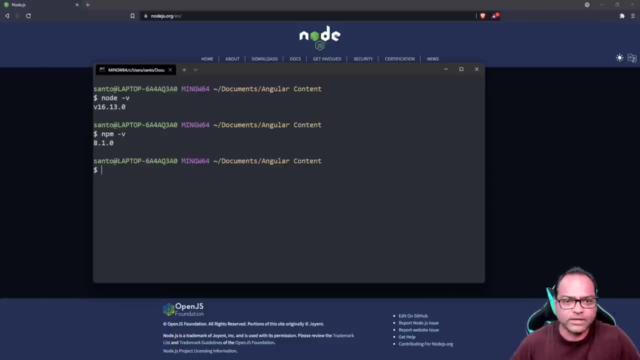 which is 8.1.0 right now, and how to use it, we will, of course, see while installing type. the next thing which we need is, uh, we need editor. as i mentioned, you can use anything, any editor you want, but we are going to see vs code. 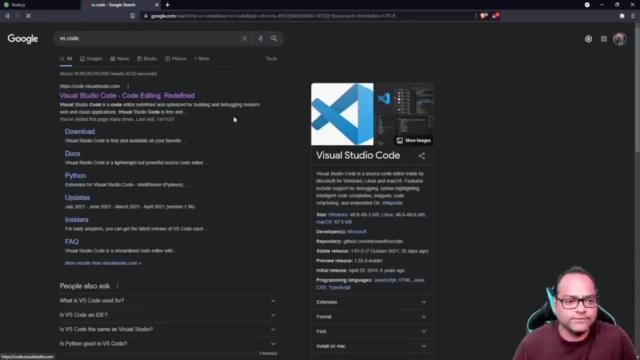 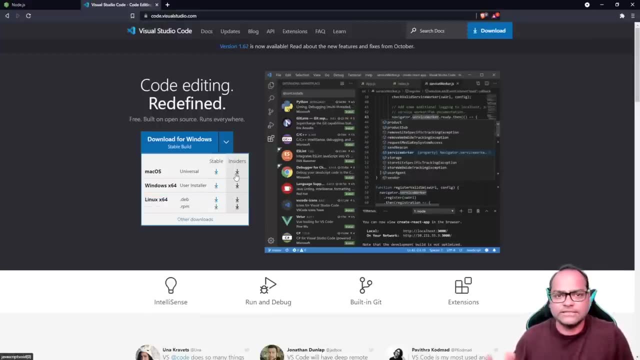 so i'll search for vs code and this is the website and you can see there are multiple versions for mac os, windows, linux. you have been stable and insiders and you may ask: okay, what is insiders? so insiders is something where uh vs code team may give you some uh access, access to some. 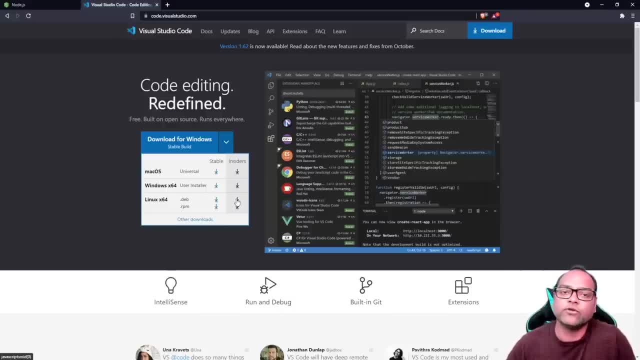 beta releases some features which is not still available for everyone, and that's what insiders is. uh, recently windows 11 was launched for insiders program first and then it was launched for general purpose. so stable is that's what general purpose is. i mean you can go ahead and 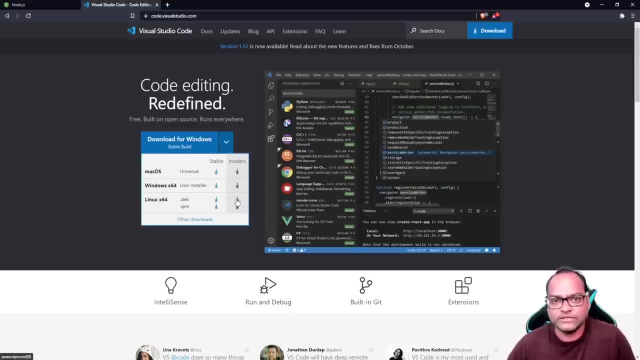 install and uh, you don't have. you get access to any beta features, but it's okay. i mean, uh, probably you will be using it in products. uh, your day-to-day development. if you're comfortable, go ahead and use insiders. otherwise, stable sign, we will be using stable and to update vs code you. 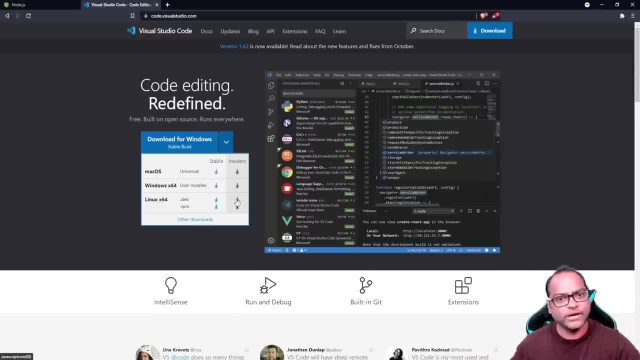 don't have to actually do it manually. uh, it's an example, but there are other features, such as: uh, we will be using stable and to update vs code. you don't have to actually do it manually. uh, it's our …. … it gets updated in background, so when, once you install it, that's it. that's the only thing which 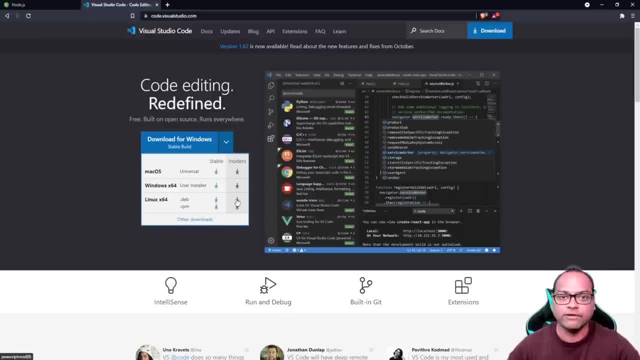 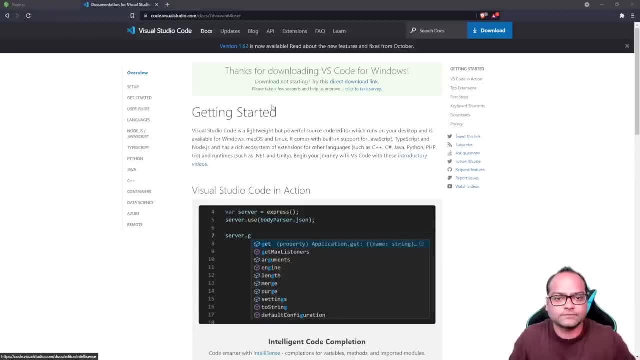 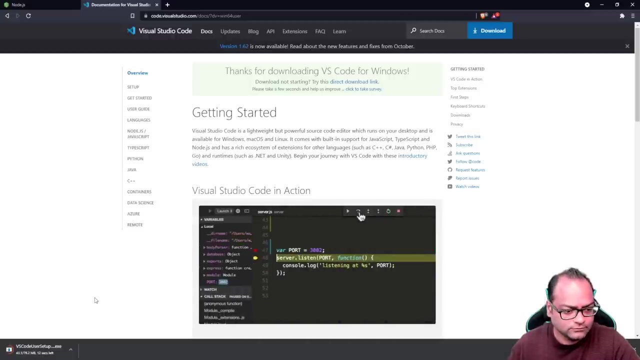 you need to install and then it will be updated in background regularly whenever there is a new release. so let's go ahead and download the stable version as of now. so it says the current version is 1.62.2. so let's see, and in case we you want to use visual studio, i think visual studio 2022 will be available soon. 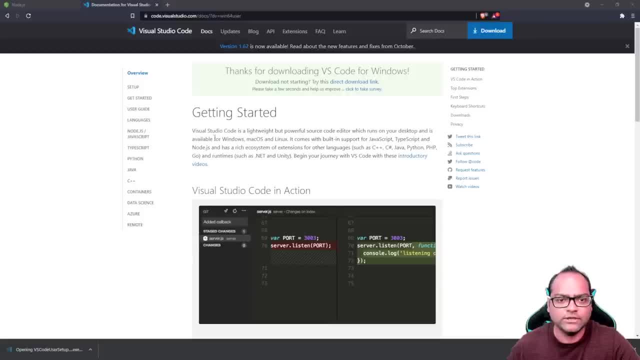 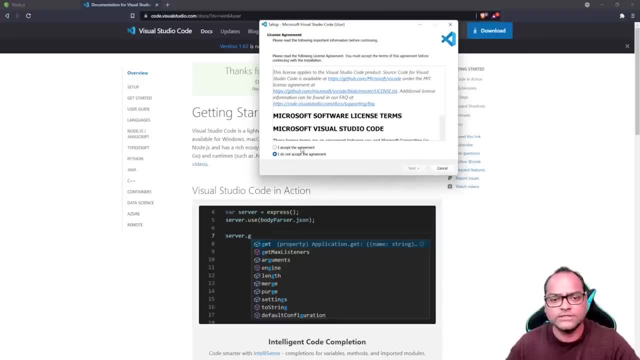 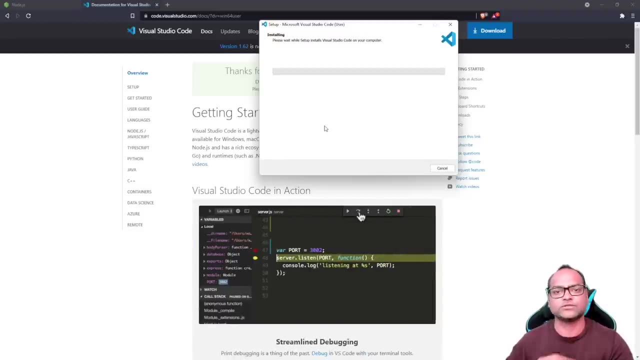 but, as i said, i don't use it. it's really heavy. you can use webstorm or any other editors which you like, so let's see. so i'll say accept agreement and create desktop icon. i'll just click on all and let's go ahead and install. i already have the latest version available. i'm just doing it. 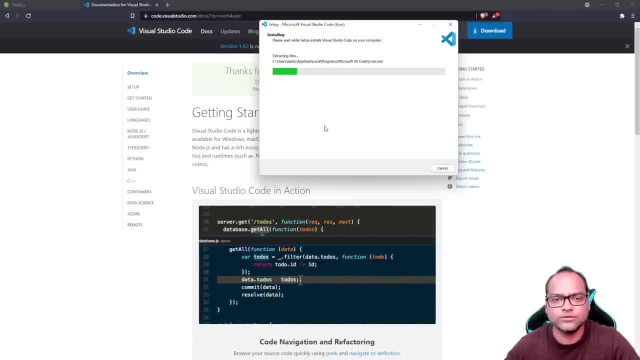 to show how to install it and again, in case you get some issues while installing vs code. generally, the problem which you get in during installation is related to the access, so make sure that you are running all the setups as an administrator, just to avoid error in case. 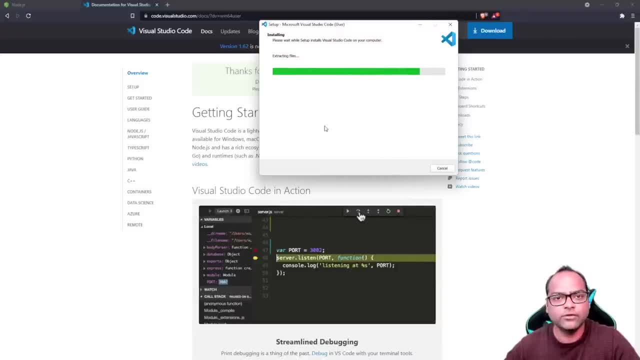 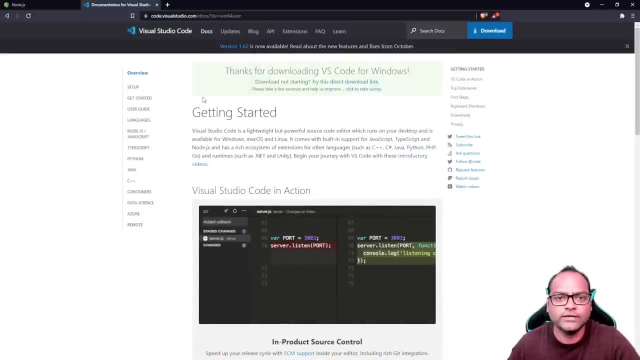 you still get some error, just let us know. we'll try to solve it before you. you use the virtual standard version, Crystal, and by the way, seems you could even use the besides version. so do like without too much use. afterimos, if this is your first gate pop up in predictions here, we will try to help as much as possible. uh, and before you. 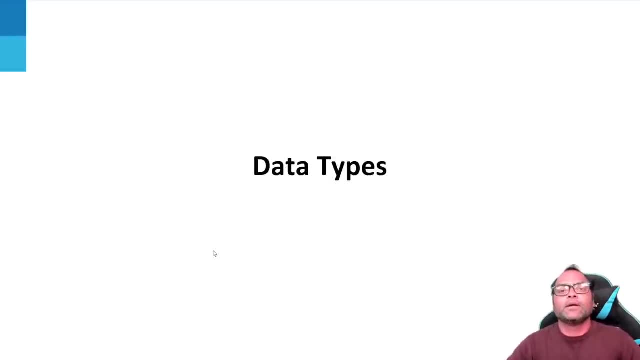 uh, like wait for the response, just uh, check it on stack for flow as well. probably you will get your solution there and that's it. so let's launch visual studio code, and we are done so in in upcoming videos. we will be using vs code for all the code which we already have. 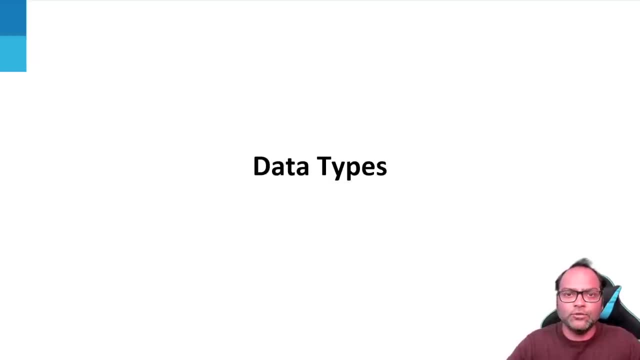 talk about data types. so whenever you start learning any new programming language, you learn about data types. i mean how, what are different data types it has and how to work with those. so that's what we are going to do now. so in data types, we will talk about data types. 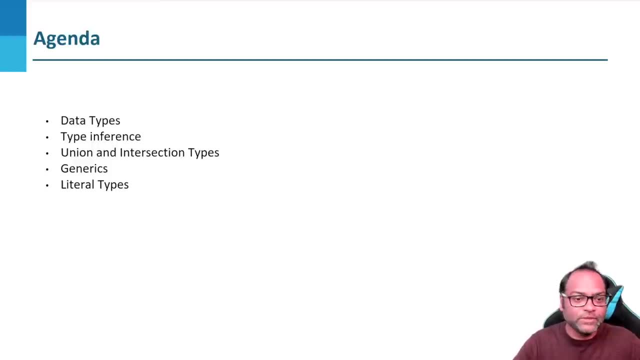 we will talk about uh, inference, type inference, which is really important. we'll also talk about union and intersection types. we'll talk about generics and literal types. so let's start with data types. so, as we said, typescript is a typed programming language and so it has a lot of 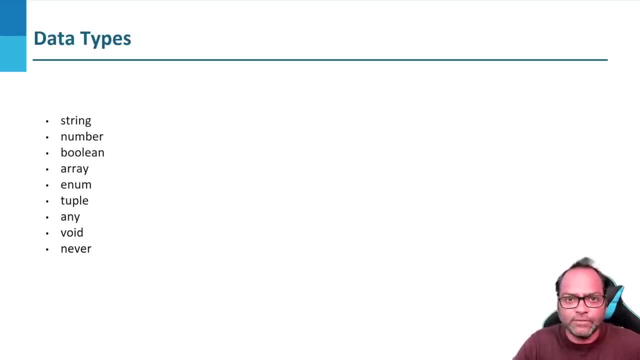 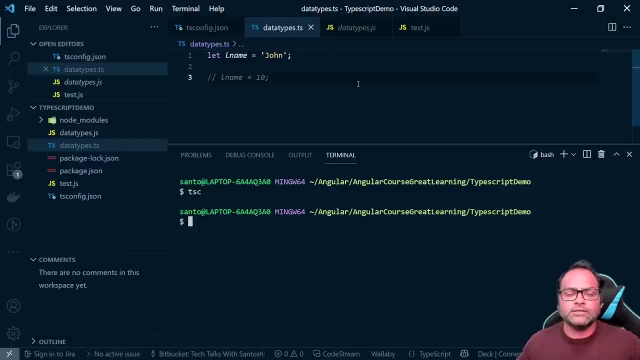 data types, which is available, and we will go through each one by one, and let's go ahead and do that. so we already have our program, our workspace, ready, and the first stereotype which we are going to talk about is string. so, if you remember this quote from the previous video, we 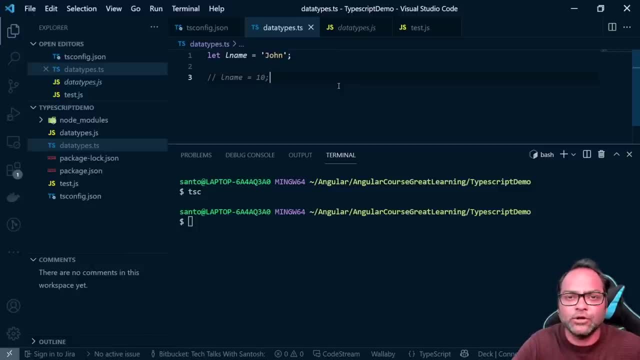 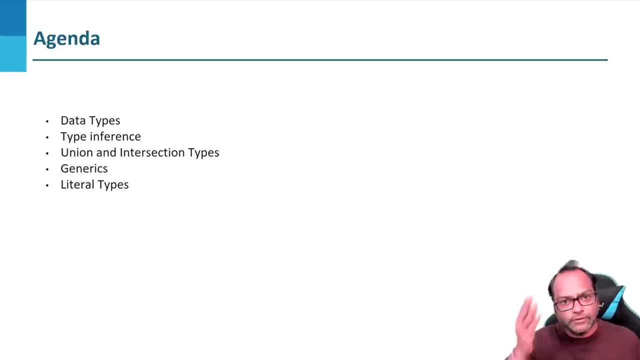 already declared something called a name and then we set equals to john, which is the string value. but how actually typescript knows that, okay, this is string, we'll come to that, but let's uh, so, let's, let's uh, so we'll talk about that. i mean, how angular, sorry, how your typescript knows that, okay, this is type of swing and this. 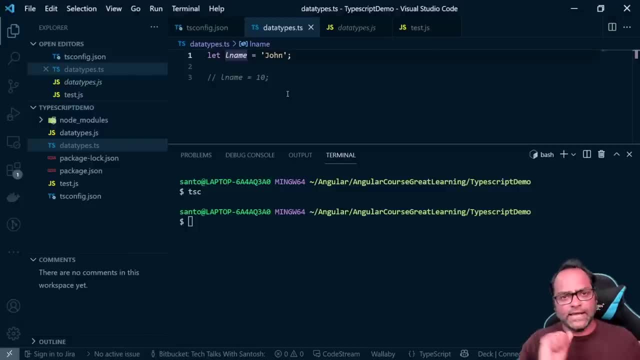 is where type inference come into picture. typescript has the ability to determine the type from the value which is being assigned. it's amazing, right? i mean you probably don't need to define the data type because typescript can actually guess it for you. but don't try to do that, i would suggest always. 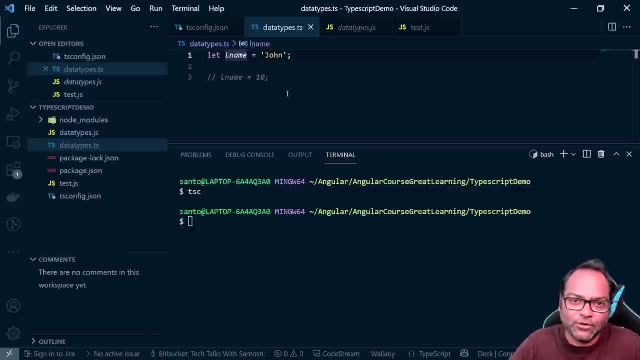 use the type because sometime, sometime, it gets it wrong when you are writing complex code and it may give you some data which is not you want. so here, uh, that's time inference, so it can actually determine the data from its, uh, the value which is assigned. so here it's a string, so it is saying 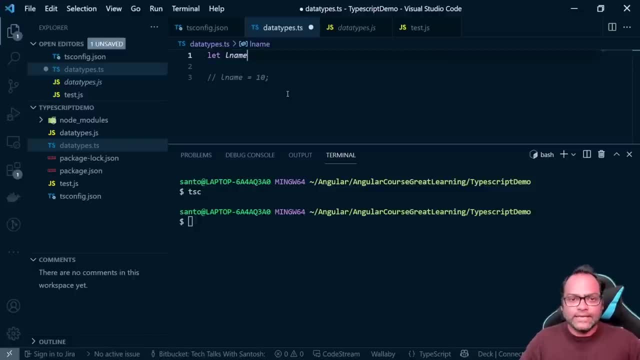 okay, it's type of string, which is okay. but in case you have to declare a new variable, this is what you will be doing most of the time. so you will say, okay, this is last name, which is type of string, and then you can assign a string value to this. so it's my name kantosh, last name um, and then 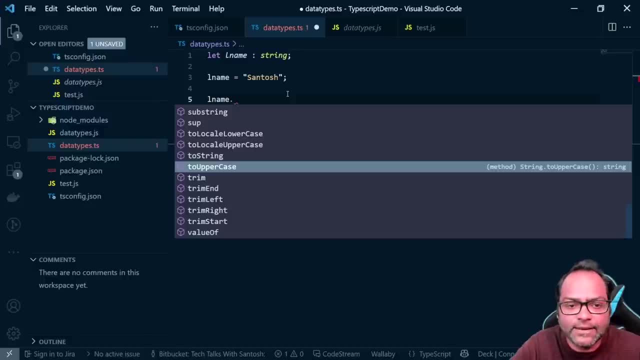 the advantage is now i can actually, if you say l name dot, generally you don't get all the methods. in case you are writing a javascript code and just declare a variable and press dot. you will get list of functions for sure, but it doesn't give you that. 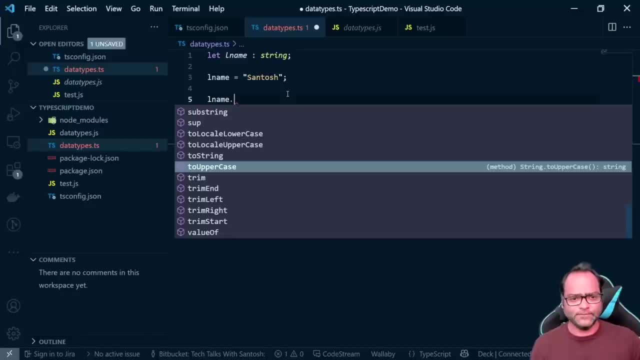 okay, this is only string function or numeric function. it doesn't give you that. here all the functions which you can see are actually uh, can be applied on string, that's it. so you have to string to string. so let's say, if i do to upper string, right, and i'll say, let 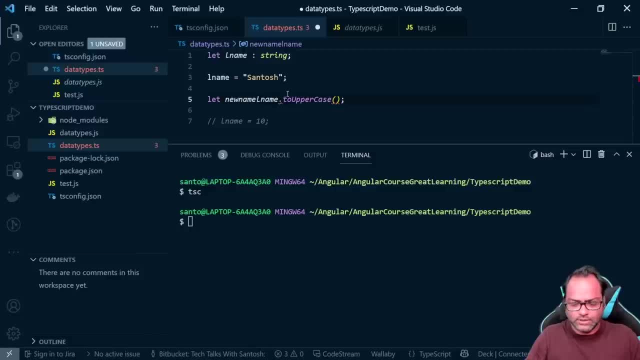 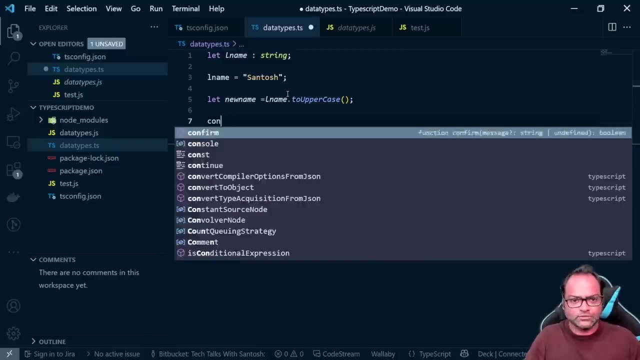 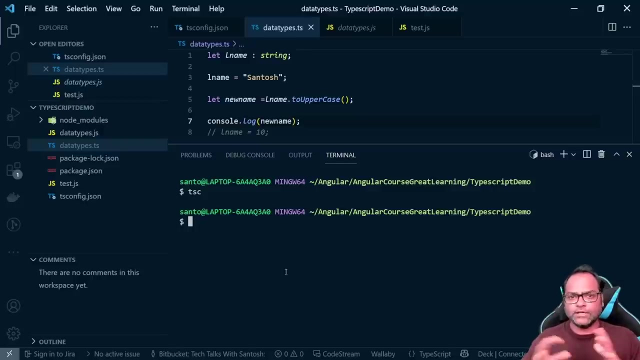 new name equals to l name dot uppercase. so i'm just updating, or i'm updating the l name to uppercase, and now let's do consolelog and see the output of this particular uh value. now, uh, here, uh, you know, type script compiler. tsc can be used to convert or typescript. the tsc compiler can be used to. 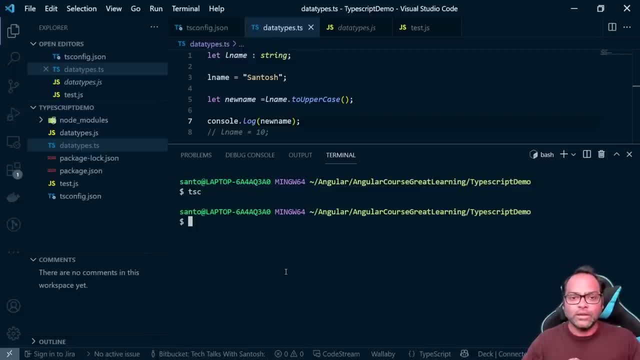 convert or compile your file to javascript code, but how you will run it. so we will be using now h, that's called tsl node, which you can also use, but we are going to use your code available here and now. i can just say node and datag. 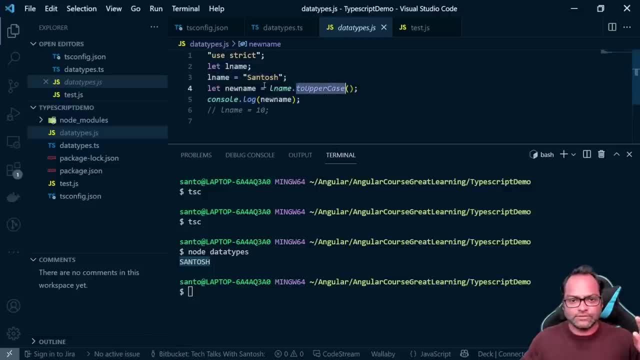 and you can see: okay, uh, the uppercase function was applied to this value, and then you have this output. so, if do, you are running this locally, because we are able to run this on my command from because we are using node node, As I said, node can be used to run your code on your local machine. You don't have to. 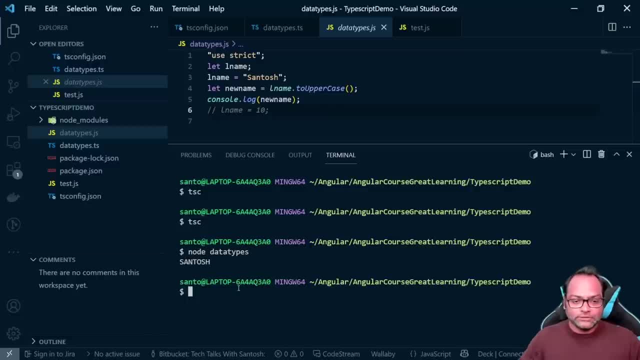 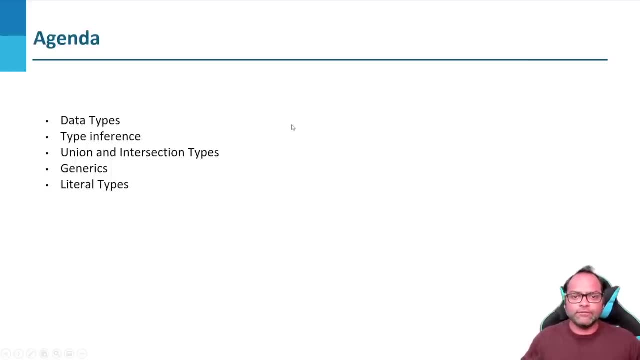 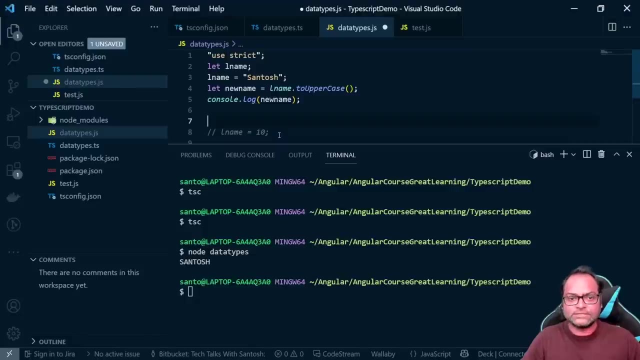 actually run the JavaScript in browser. So this is string. I mean, let's see the next data. So it also has something known as number. So let's talk about numbers. So whenever you have some numeric value to assign, go ahead and use number. For example, let's say let age. 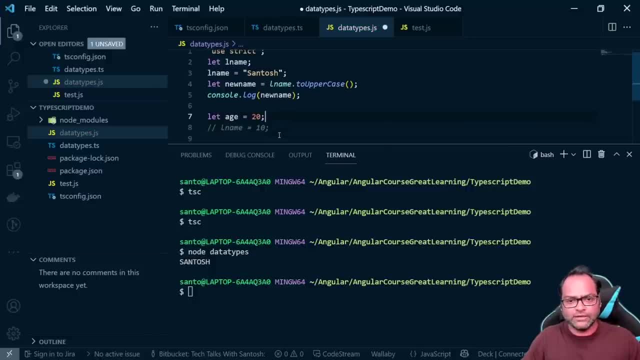 equals to, let's say, 20,. right, But you can do this because of type inference thing. But in case you have to create a variable and you don't have a default value, you can say type colon number- Sorry, not the N capital, but yeah, lower. So you can see it says: okay, now you have. 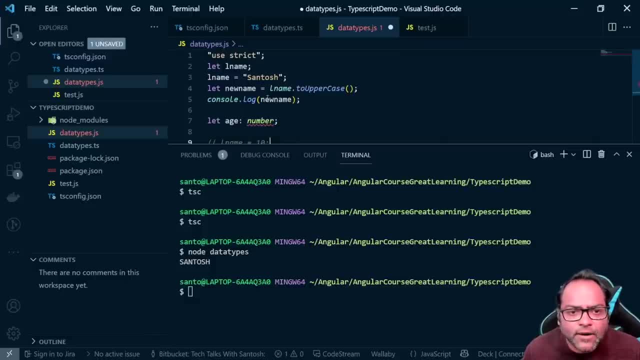 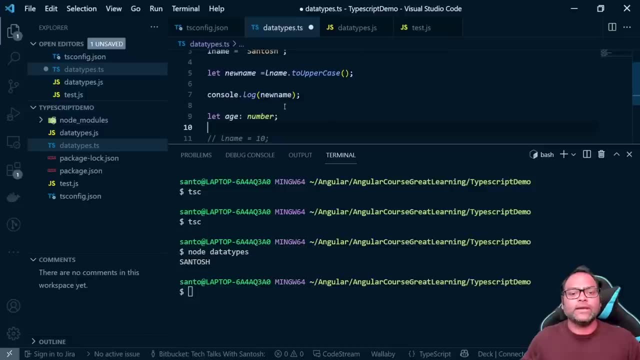 let age. Okay, I'm writing code in JavaScript 5. Not bad, And you can see, I can say let age, which is type of number, And now I can say age is equals to 25, which is a value, numeric value. But if I say age is equals to 25,, 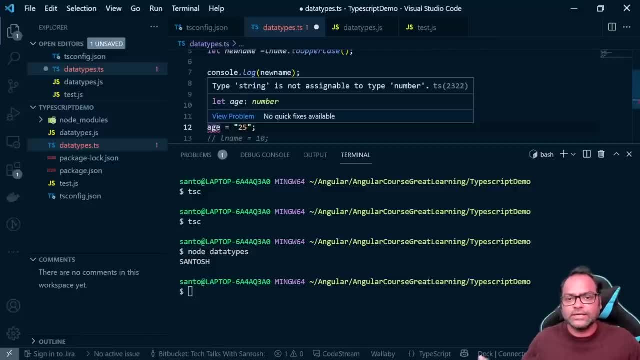 it will give me an exception. It will say, okay, this is string, but I'm expecting number. So, yeah, this is something which you can do. You can also do decimal numbers. So, in in case you have like decimal numbers, you can say 25.5.. That's also applicable. 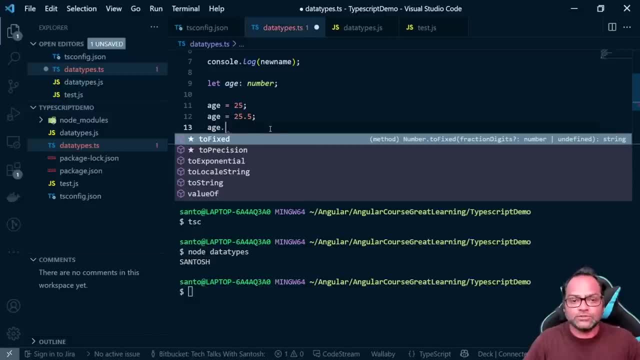 That's, and you here right, So you can see age dot, So you can see, you will be only able to see the function which can be applied on numbers. So you have to fix to precision. but what in case? let's say, you want to type cast, which happens right Sometimes. So 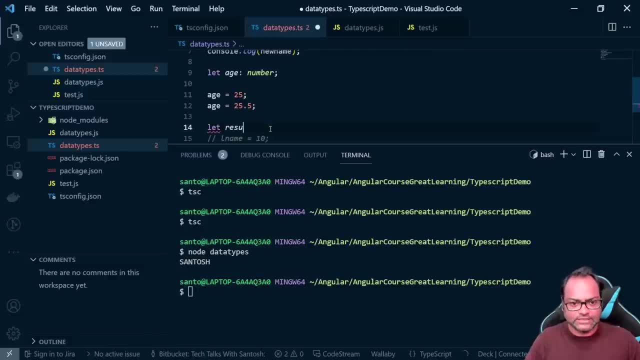 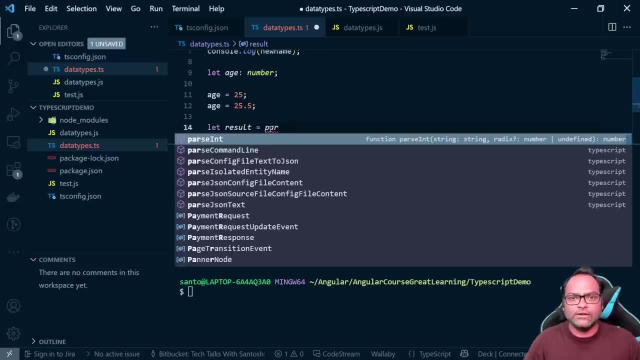 yes, that's, that's possible as well. So I can say: let result equals to. so let's say, if you want to, you have a numeric string value and you want to pass it to it. This is a normal JavaScript function. This is something which is not coming from TypeScript yet This is something which is: 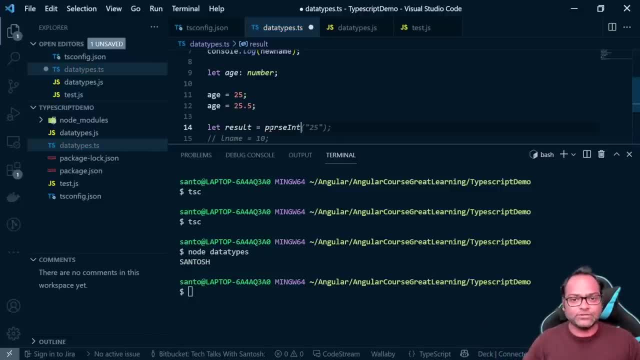 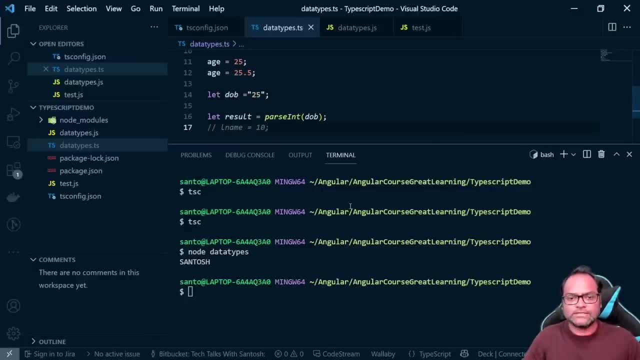 you can pass the string here and using percent you can convert it to number. and let's see the magic here. So it says result will be type of number because, as I said, due to type inference functionality, TypeScript knows what, what will be the return type. So percent returns a number. 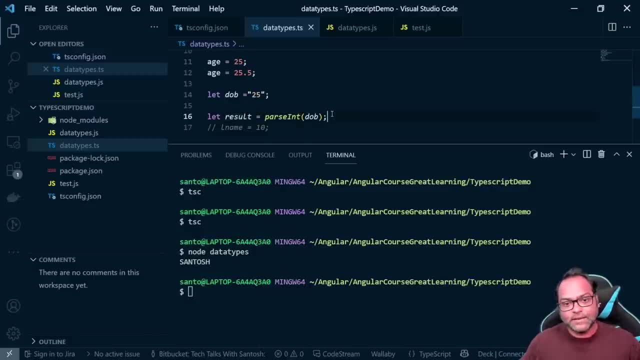 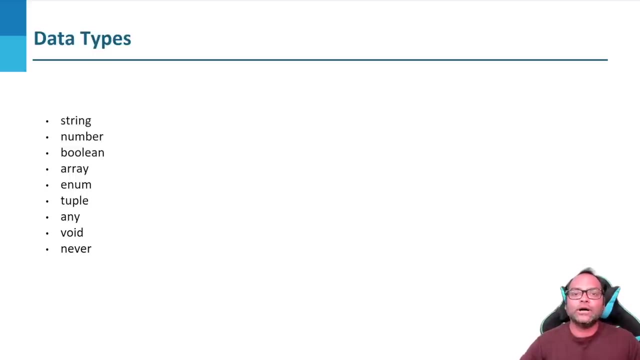 and that's what. that's what the output is. We will see some- I mean, we will see functions as well, where we'll, of course, try to play with this- data types, and let's see the next. So, after seeing a number, there's Boolean as well, which is available in almost in most of 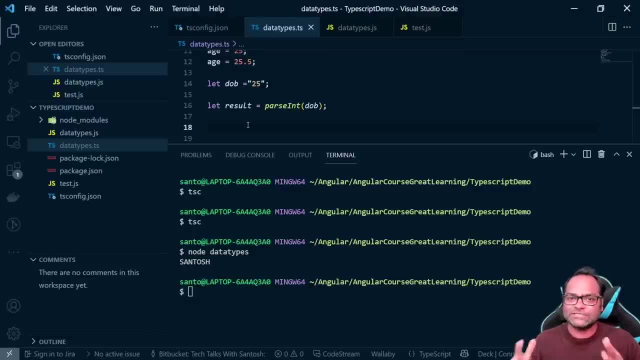 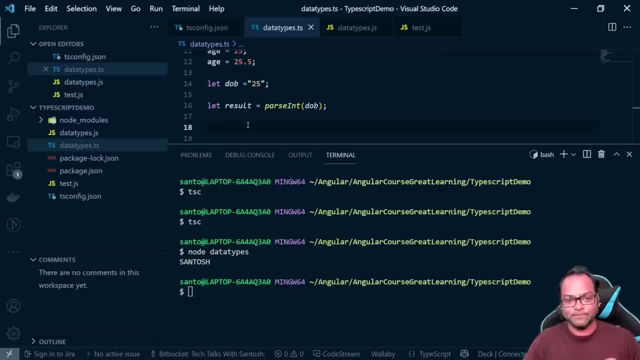 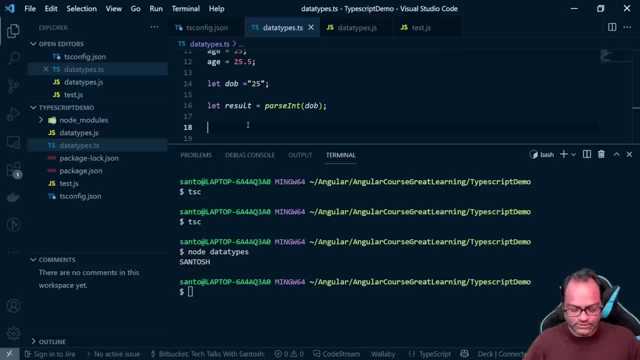 it has a default value, It's false, right? So let's see. So select is valid, which is type of Boolean, And in type safe language like NET, in Java, we have habit of doing. this is valid of type Boolean because we know, okay, it will return the default value as false. but let's see what. 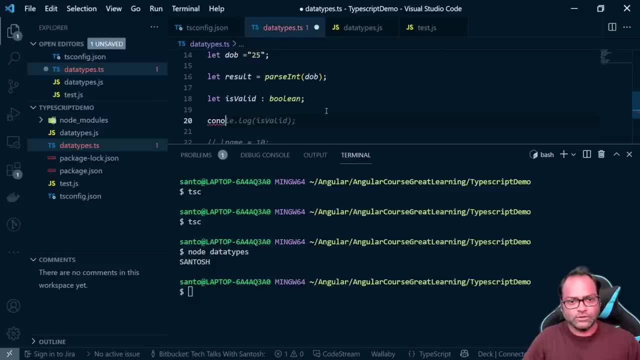 happens here. I'm going to do consolelog: result And not result is value. sorry, And you can see here there is one error. So it says variable is valid is used before being assigned. It is telling you that, okay, this value is not assigned. 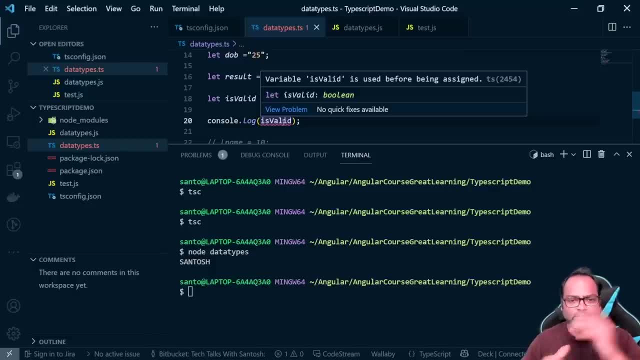 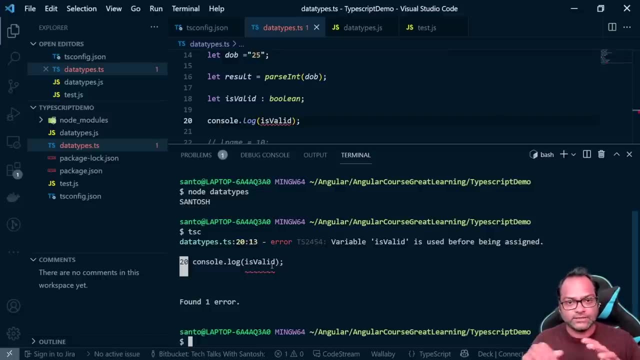 and it is just giving you a quick warning here. But let's see, let's see what happens when we run the boot. So I'll say TSC. It will, of course, print this warning here and this error. sorry, It will print this error here as well. 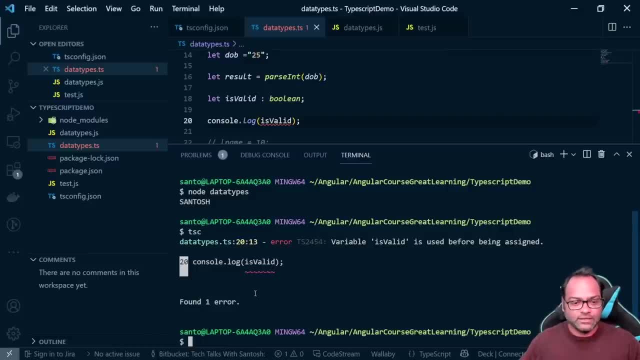 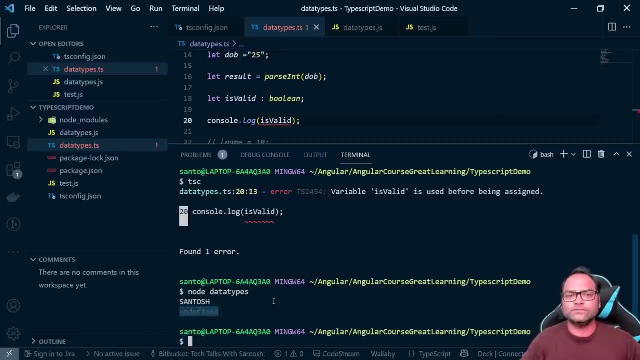 And why. I'll just come back to that in a second. But let's run the node and data equals And you will see you will get the value as undefined. So where is the default value gone? So actually, just let's go back to earlier video. 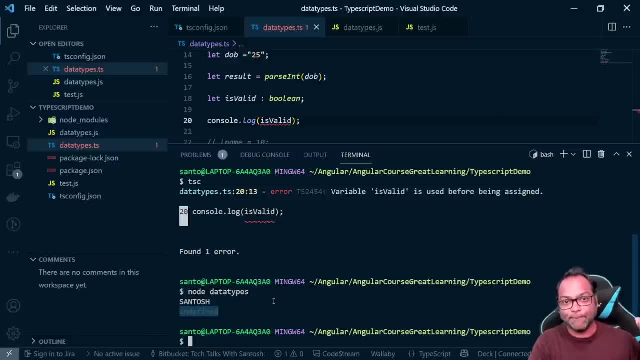 where we said that Java types will be compiled down to JavaScript. JavaScript doesn't know anything about types. So if I go to types, stereotypesjs, you will see is valid. that's it. And if you write this code in JavaScript, it will be undefined because you have not assigned any value. 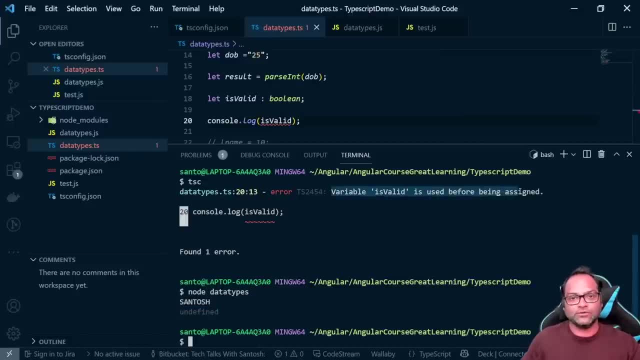 That was the error, which is printed here. So it says it's not assigned. So of course it was expecting that it will fail. You have, you're trying to access a variable, but you have not assigned the value, so it will be undefined. 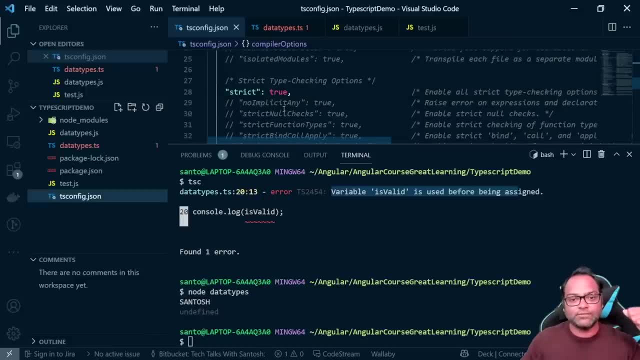 Why we are getting this error? Because of tsconfig And there is a property called strict true. So if you keep this in, if you use a district mode by default, which is by default, you cannot or you can, but you will get an error. 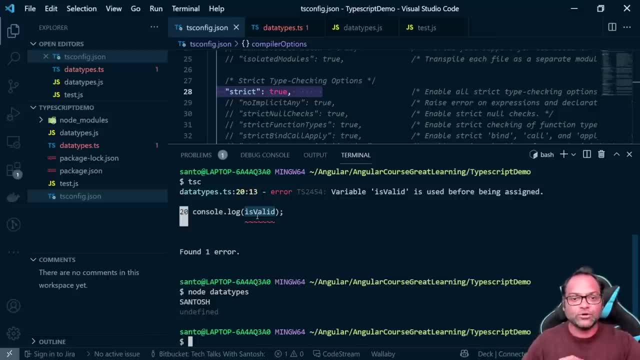 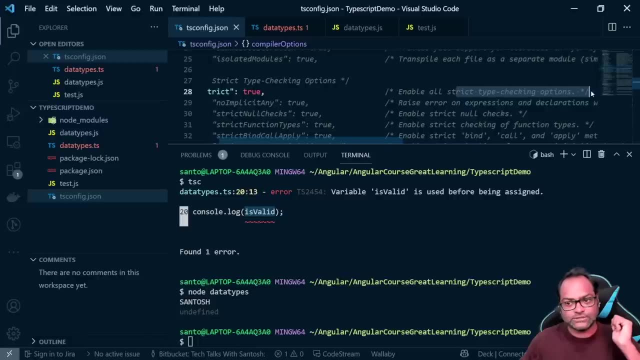 if you try to access any variable which is not defined. So, while working with TypeScript, keep district mode true, So it's like it enables all strict type checking options. So you can see it says enable all strict type checking option. we will discuss about few of this. 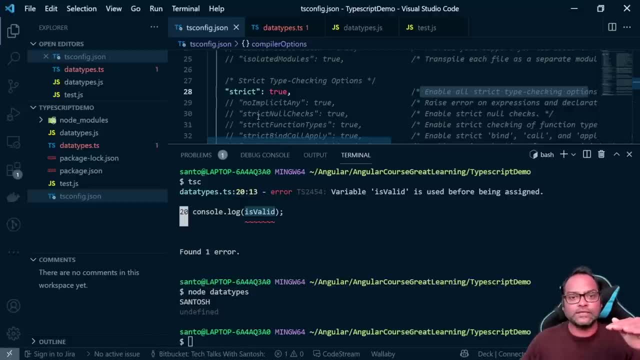 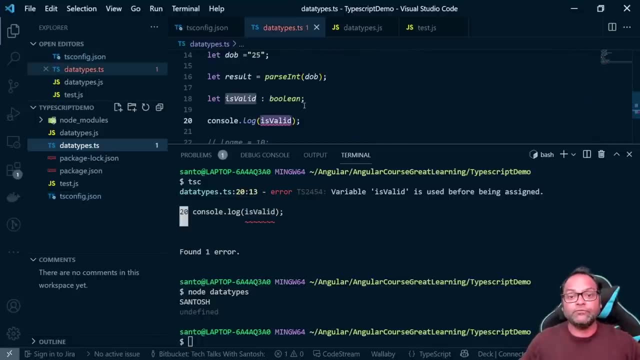 strict type modes, but right now let's go with the strict mode, I mean, where all the strict options are enabled. So yeah, that's why it was giving an error. So whenever you are working in Boolean, make sure you define the default value. 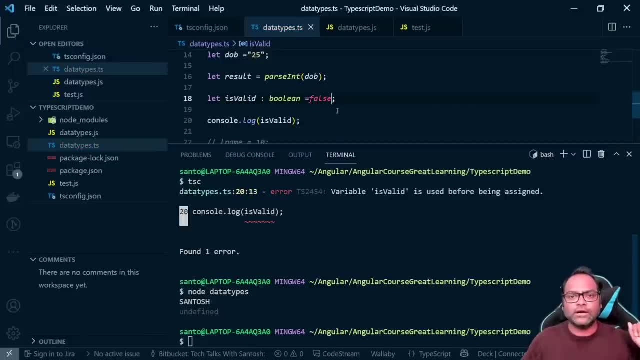 So either true or false, whatever you prefer, I mean whatever fits, of course, into your workflow or in your code. So use default value false, alt, alt, And now you can see the error is gone itself. So you might have seen one more advantage. 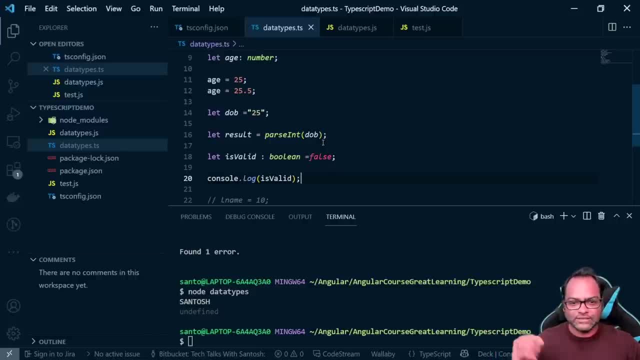 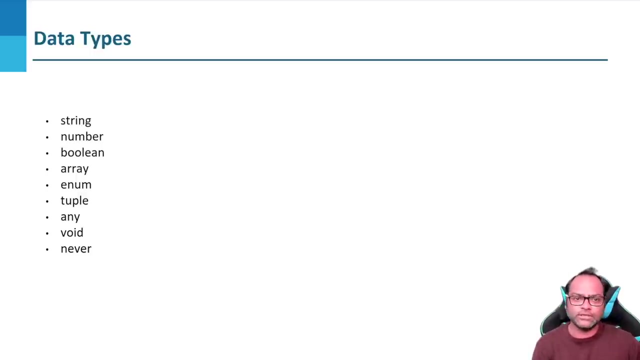 Is that you don't have to actually most of the time run the code. You can actually see this type related error inside your terminal itself, So it saves a lot of time during the development. Now let's talk about the other data type. 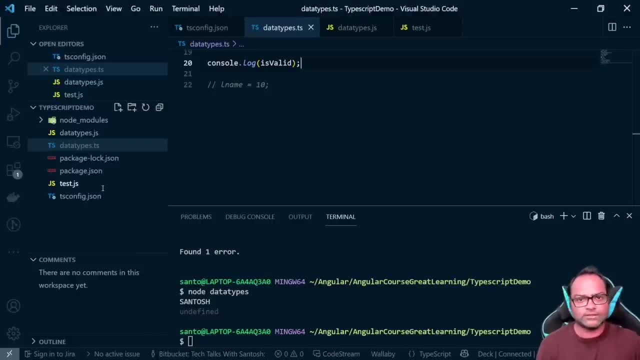 which is the array. Again, I will go back and refer, for example, NET or Java, where you have list types available, right? So you have list which is available in type in Java as well as NET. In JavaScript world we use arrays. 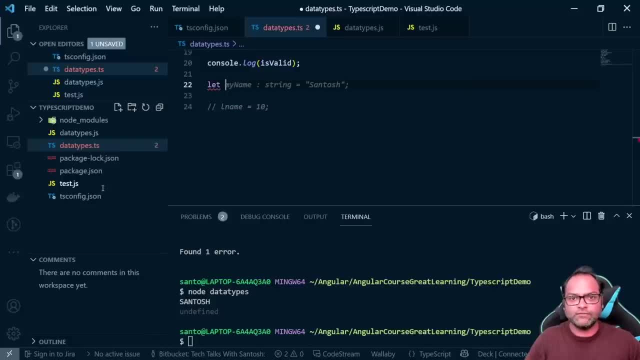 and generally we do something like this. So let's say: if you have amp-list, this equals to this. This is generally how your array looks like in JavaScript. So here if you see the type, so let's say it says any of array. 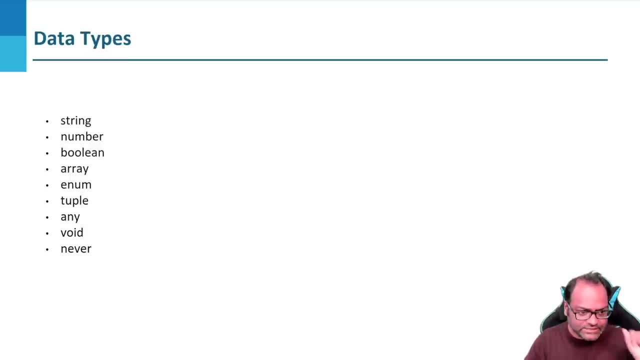 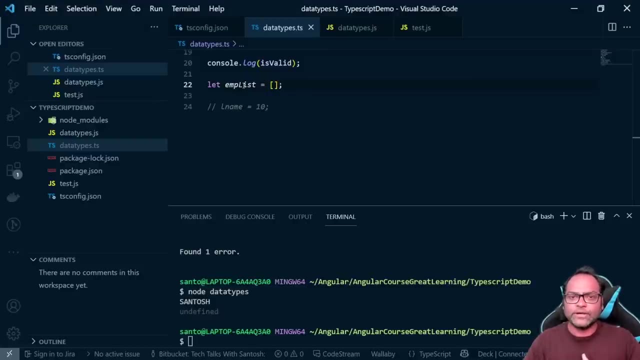 What is any? So if you see here in the data types list, there is any as well. So we are going to talk about any. Let's come back to that later. Let's talk about arrays. So in TypeScript you can declare a variable. 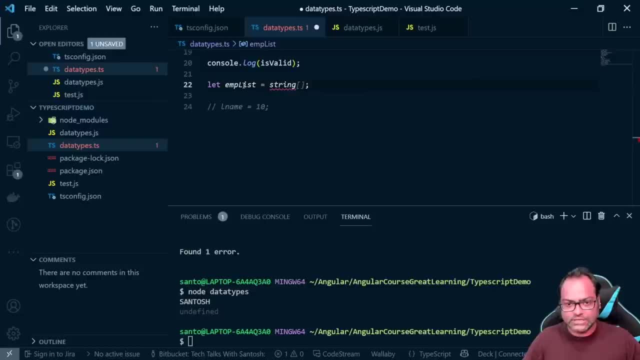 as an array of some data type. So you can say string array, For example, if I just want all the values, sorry, I want this array to only hold the values of type string. what I can do is I can say string and then box. 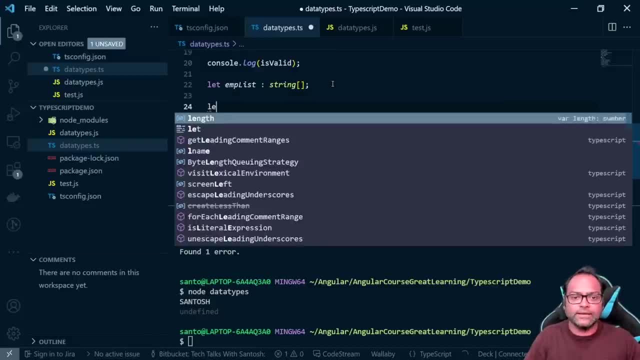 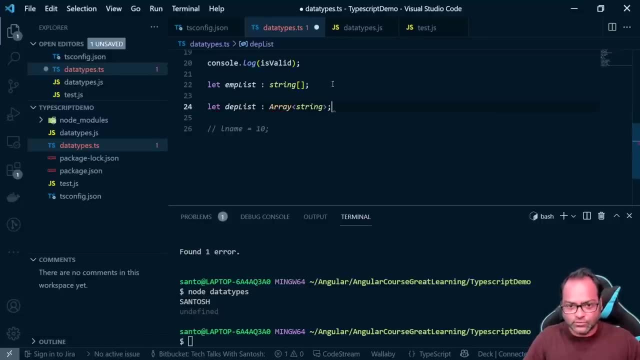 There is another syntax which is available as well, So I can say, let I can say, against a department list, which is: you can also use this syntax which is known as array, and then you can use this rectangle boxes. this is known as generics, so that we will also talk about genetics. 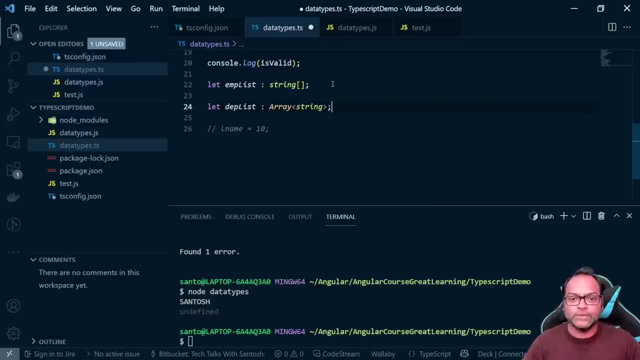 and uh, we will also talk about generics, but as of now, let's just see the syntax. so yeah, these are two ways in which you can define an array. feel free to use anyone. so it's same, because once it is compiled down to javascript, you don't, you will not have this particular types, right, it will be. 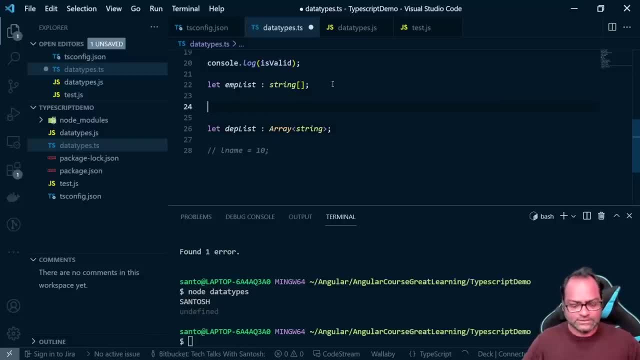 removed and then, uh, let's see, i can say emp, list is equals to. i can create some arrays and i can have string right. so if i try to add a number, you will see: uh, i have, we have an error. so it says number is not as unable to type string. so 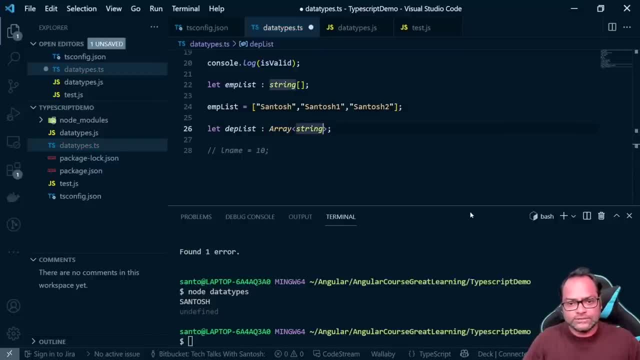 yep, this is string array and let's change this to numbers list and we can say number of array, of number, right, so i can just hold numbers here. uh, let's create a number list equals one, two, three, four, five. these are five numbers. there are few functions which you can apply. i will, i will talk about few functions as of now and then we'll. 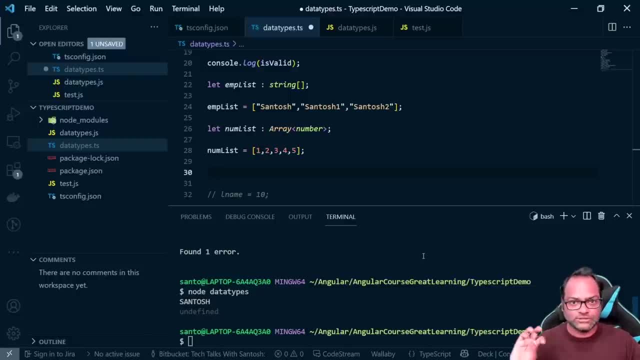 talk about few functions when we talk about interfaces, because, um, you can do a lot while with interfaces. so here let's see number of arrays. so here you can see num list. so let's try to use some function right, which we generally use in javascript. so here, uh, let's try to filter all the values which 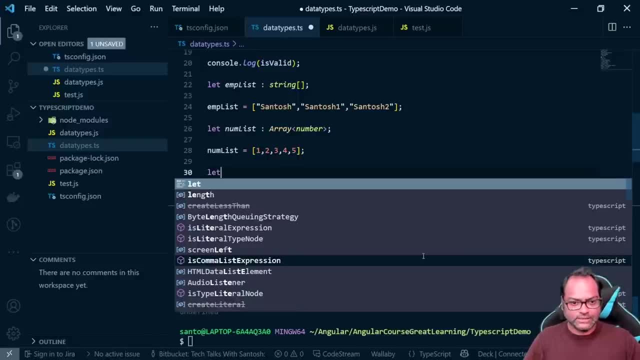 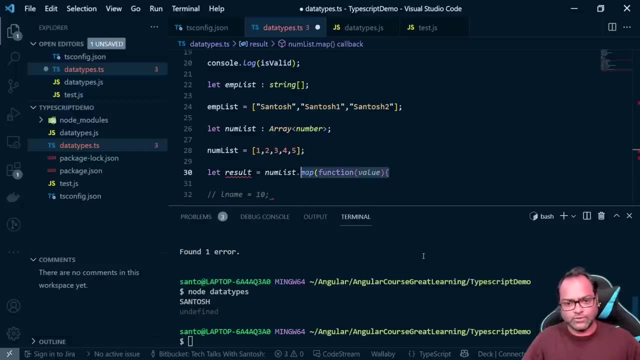 is greater than two. so i can say: let result is equals to. i can say: num list. i'm not using my, i'm not going to use map, but i'm going to use some uh function called filter. okay, so this filter function. by using this filter function i can say: okay, each number. 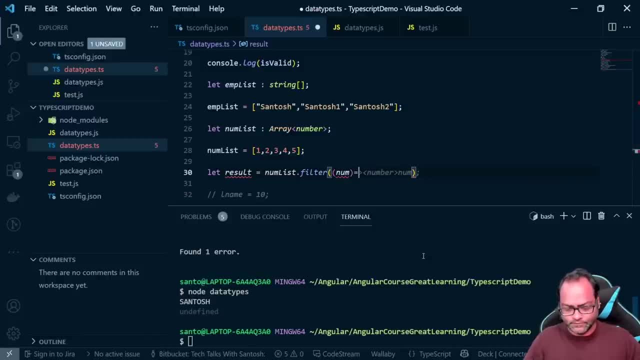 i'm accessing each number and then i will say: uh, num is greater than two and this is closing. so let's see, uh, here, uh, i think result is already declared above. that's why it is giving me error, so i can say results and i think this is extra. so now here, let's see. 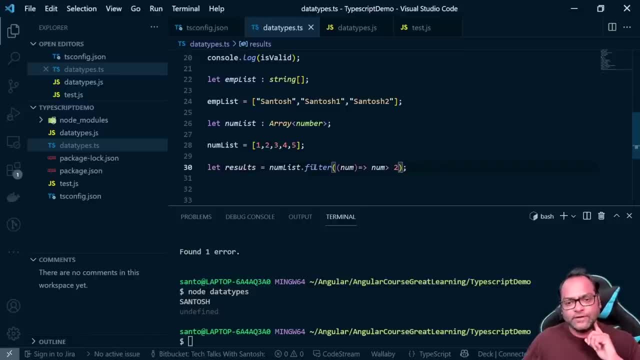 the output. so it says: okay, result will be number of array. so this filter function, which is, of course, uh coming from javascript, it's same, it uh. here what we are doing is we are filtering all the values within this array where number is greater than two. so if i print this output, 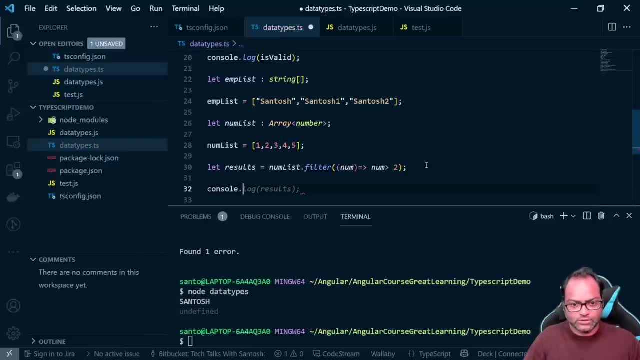 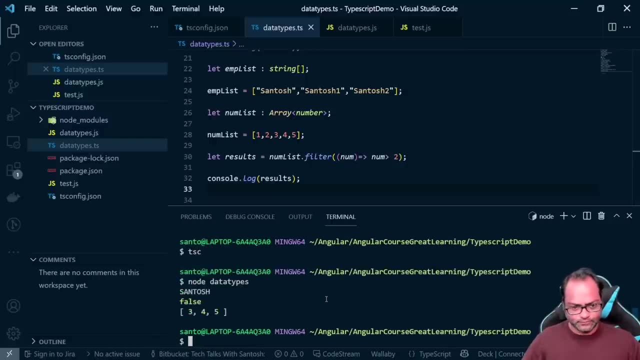 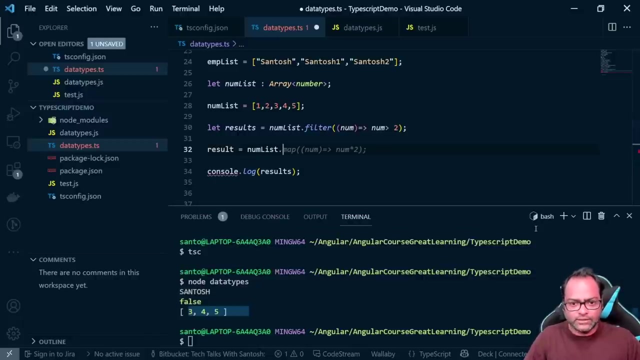 i can say: okay, the system is so: dot log results and let's compile using touch compiler and then run node. you can see: uh, we have output 345. also we can use few more. so i can say: results is equals to i can. let's use some other function and find. let's use find. so i want to find a. 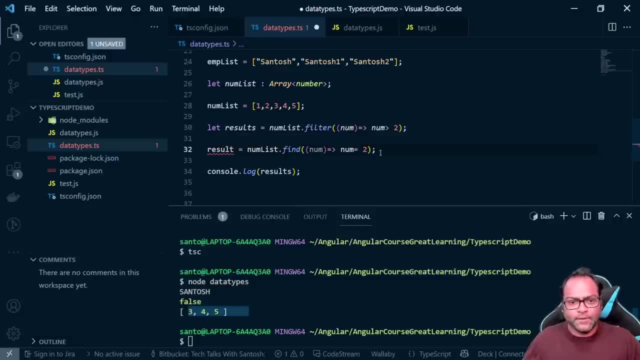 number which is equals to. okay, so here there's a catch. so if you see this results, it was expecting number of array here. if you see this, it says number or undefined, because, uh, find method returns only one value, so it doesn't return an array. so just that's why we are getting that error, because, 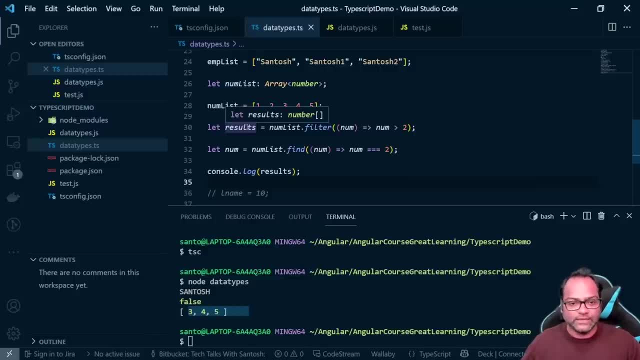 array. it was array and then we cannot assign it number, so that's not possible. so i can just print console dot log number and you will see that we will get the number. i mean of course number two. number equals to two which exists. so let's see: uh, we have. 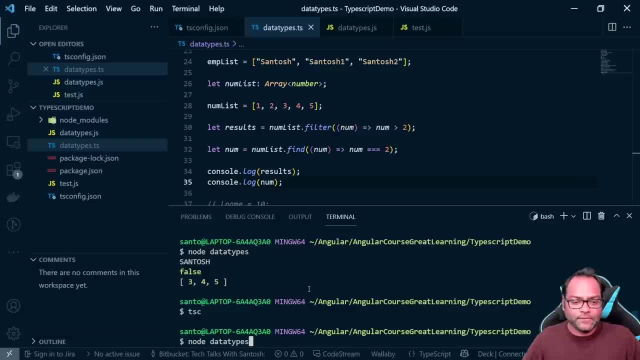 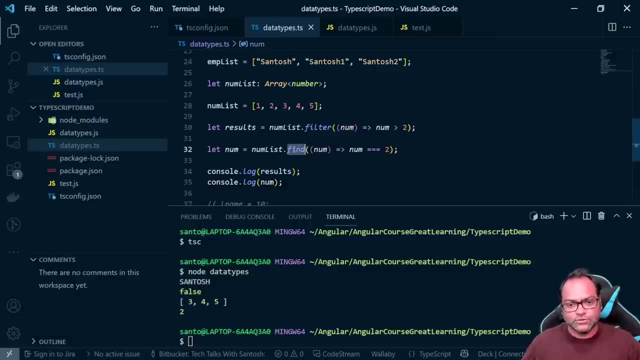 and then node. So of course two is available in the array and we get that output. So this is find. You can also use find function in case you are trying to find a single value, For example, let's say this: employee: right. 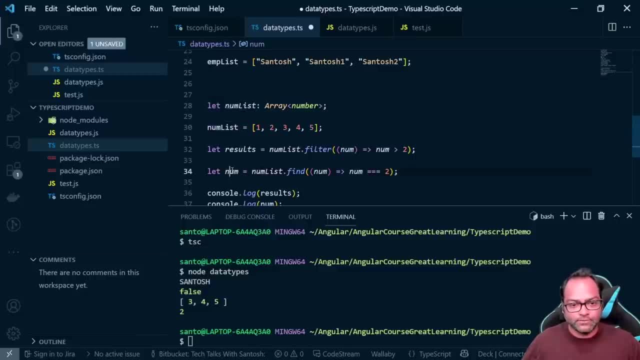 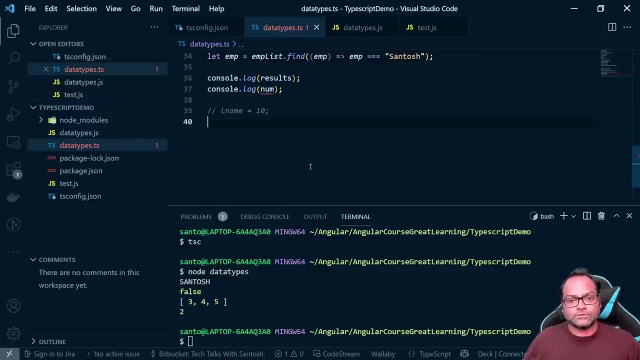 So I think that's the best use case where I can say if this employee exists or not, right, I want to find that particular employee. So I can say EMP list, dot find. then I can say EMP, and then equals to EMP, goes to this and then select. 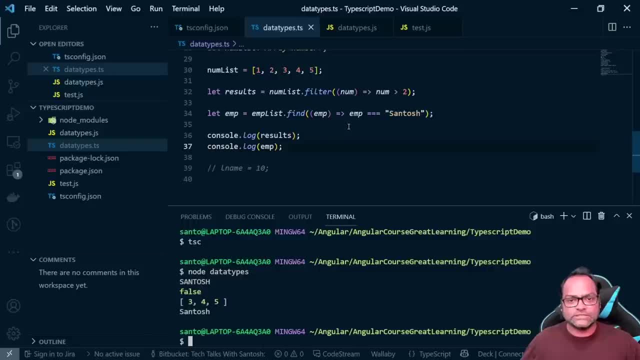 And then we can then node and then we found that particular value. So this is how you can use, find You can also. let me show you a simple example of sorry. let me show you another example of reduce function, which you may have heard about a lot in JavaScript. 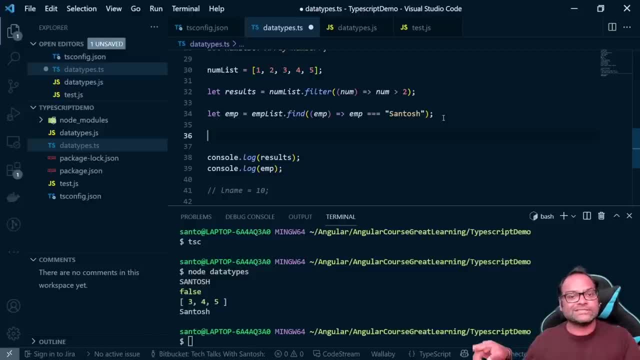 how you can use it. So I'll use it to calculate the sum of num list. Let's see. So I'll say: let sum is equals to, you can see. I mean, if you can see this magic which is happening here. 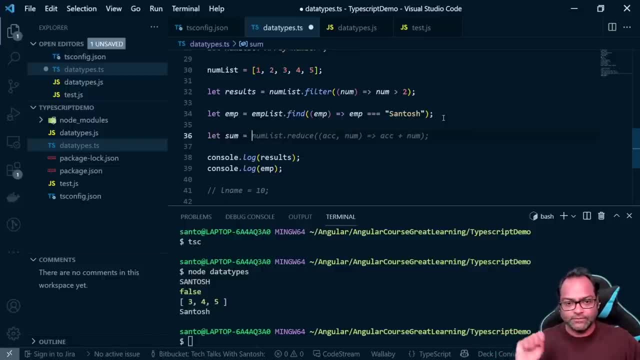 this is something because of GitHub copilot, which is a product by GitHub And right now it is in beta and you can apply it for wet list, So you can also use it. So it says num list dot reduce, So this is reduce function. 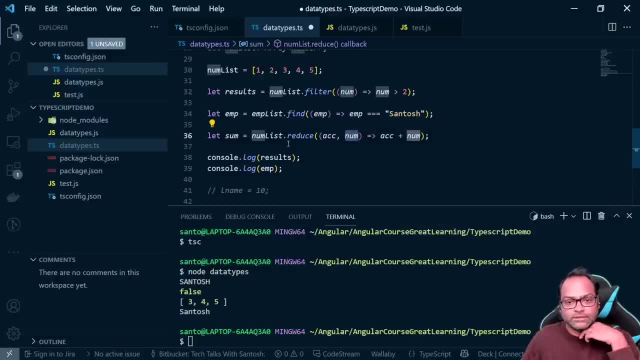 And here is a accumulator and the number. The way it works is it will calculate the sum till it reaches the end of the array. So let's see, And I'll just do console dot log sum. So the output should be one plus two. 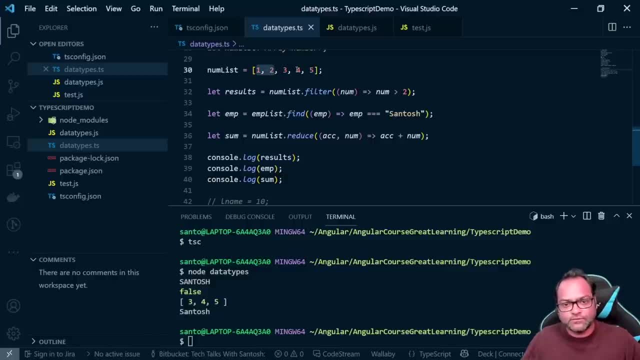 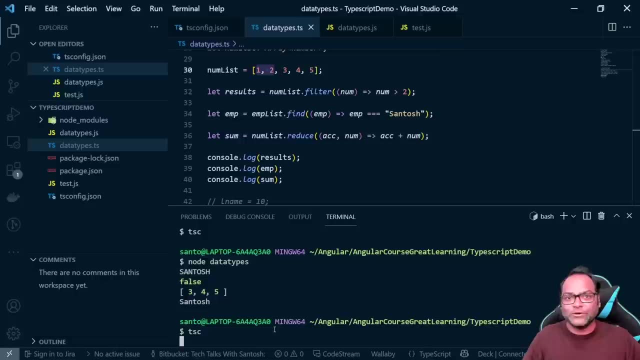 which is three, then three plus three, six, six plus four, four, six plus four, 10, and 10 plus 550.. So let's see if I'm right, I mean if I'm good at math or not. 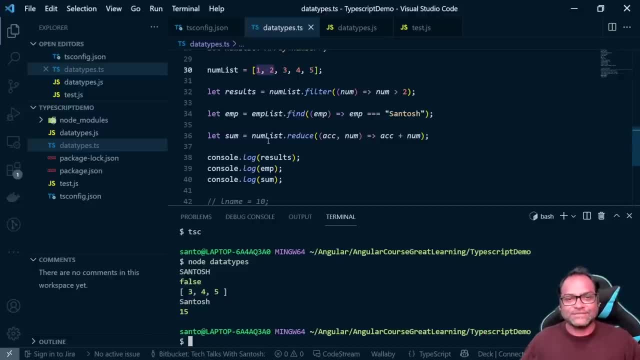 So let's go to node and 15.. Oh yeah, So I am good at math. Just kidding, It's a simple math, So yeah. So this is how you can use reduce function to actually go through entire number. This is reduce is really useful. 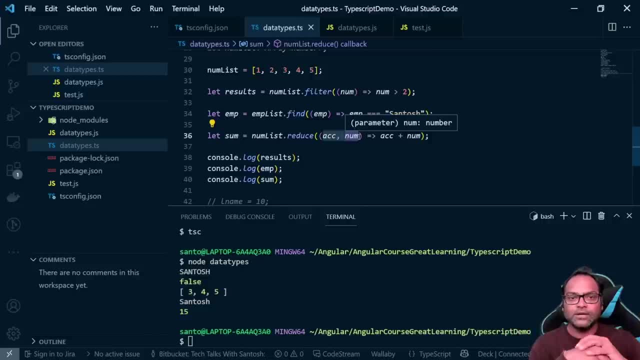 in case you have area of some object and then you want to calculate. let's say you have products right, And then you want to calculate the sum of your card You can use reduce. So these are few functions And we, as we said, 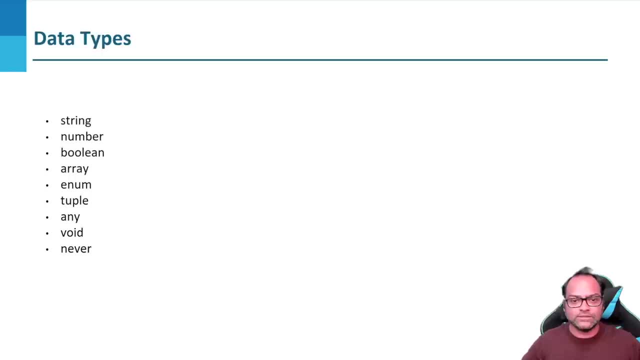 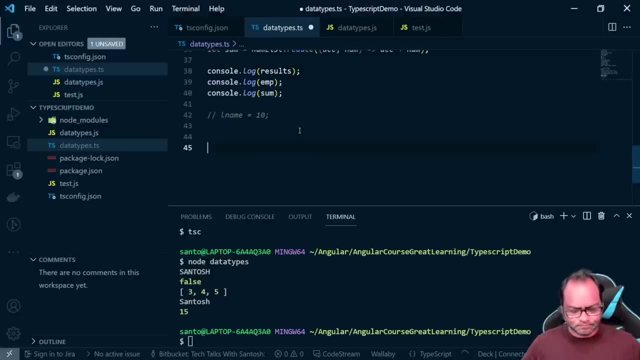 we will come back to the arrays when we talk about interfaces. So let's move on And let's talk about the other data type which we have. This is enum. Enums are really handy and it is available in most of the programming languages. 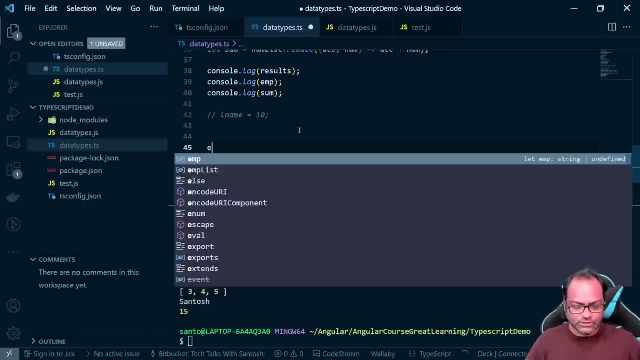 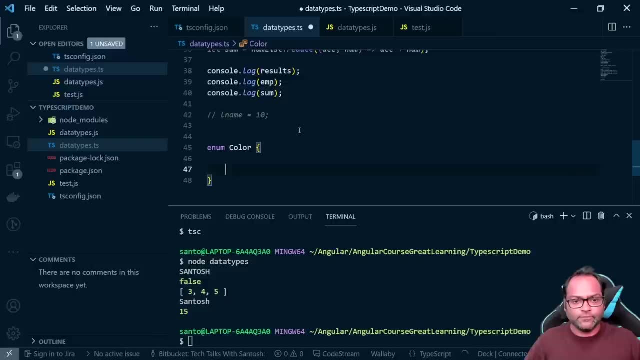 which we use. Let's see how you can actually use those. So here you can use enum, and I'll take a classic example of color. So let's say I have a enum color and then what I need is red, green, blue. 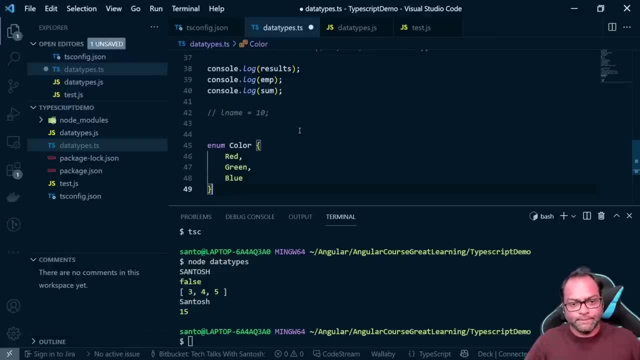 So red, green, blue. So let's say, you have some- probably- design system where you want to restrict the colors which your team can use. What you can do, Of course, you can give them the list of colors that okay, these are the colors which can be used. 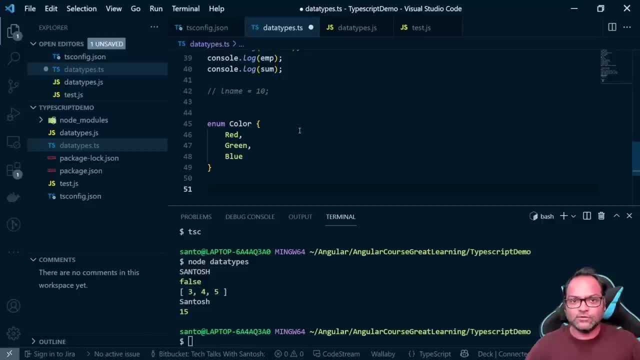 What in case? you can give them a typed list. of course, this, this is enums, right? So you can give them enums and you can say, okay, these are the colors which can be used. So, let's say, if I want to create a new color, 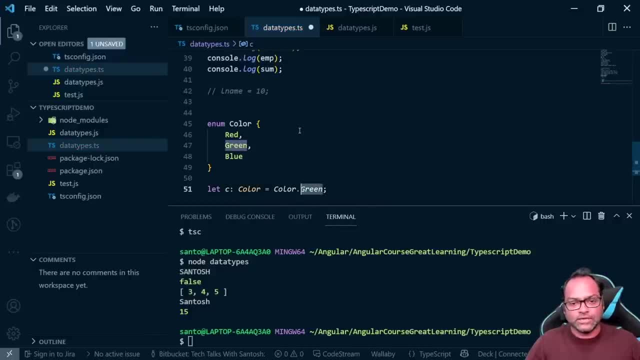 so I can say C, which is type of color, and then I can choose color dot and I can say: okay, which color I want: green, blue or red. So this is how you can use enums. Let me show you a magic. 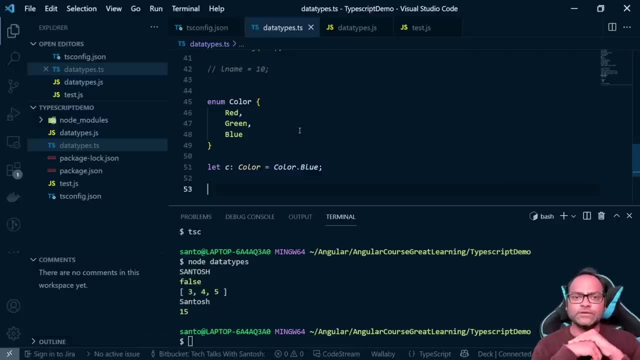 As I said, right, as I said in previous video, that whenever you compile down your TypeScript, these types are actually- I don't know- actually removed. They are not used. That's only until you write the code, And with enums, in most of the cases, 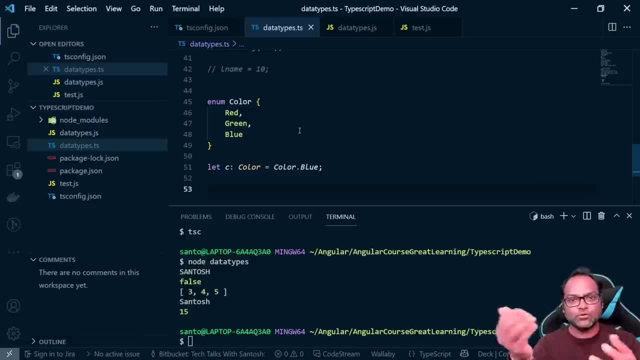 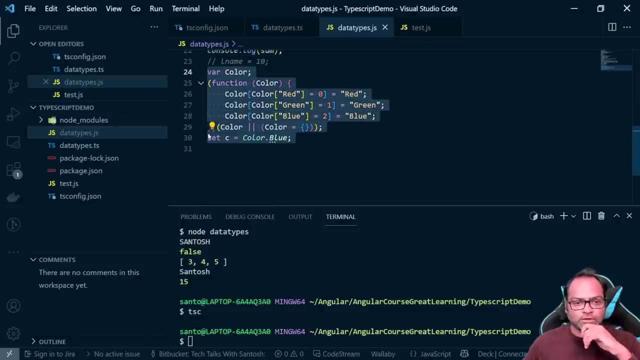 you are not going to use enums on production. I mean, once your code is compiled, you won't need this enums. But let me show you what happens when you do DSC. So this: how many Six lines of code is actually generated for that enum? 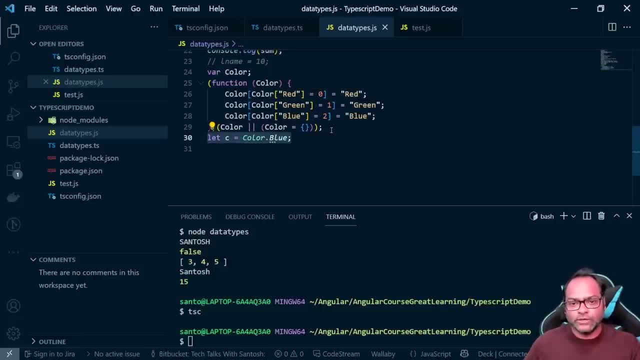 But on production, what I need is this line. I don't need to know about this, because of course I cannot change this value once in production, right, Once my bundle, once my code is compiled. So how to take care of it? 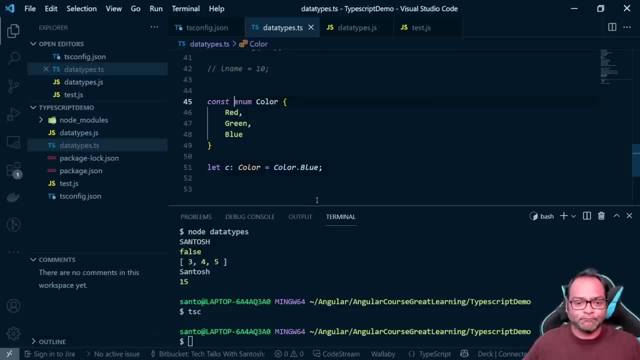 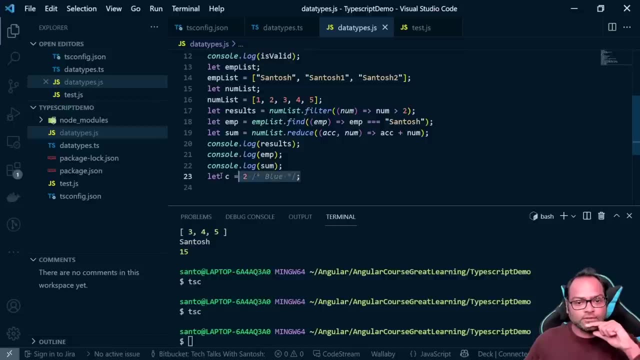 TypeScript allows you to declare enums as const, and this const will do the magic. So let's see what happens. That's it. C equals two. that's it. This is the code which will be available on your production. So what this const will do is it will just trim down. 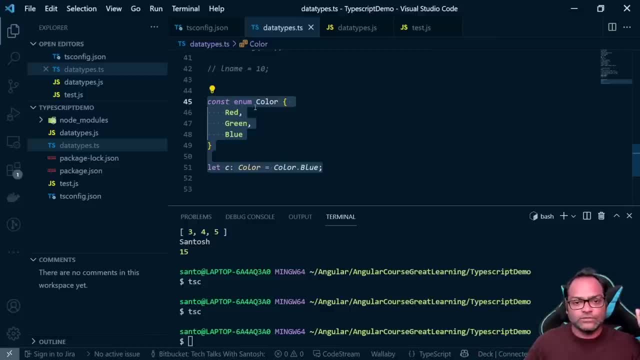 everything. it will remove all the information, because if you see enums, enums actually have an index value. So you can see here: zero, one, two. So it will just keep those index values and that's it. It will trim down all the type information. 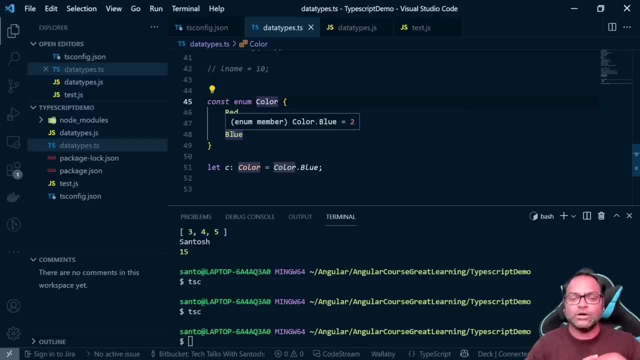 So, in case you are not going to use this enums values on your production, remove it by using, by declaring them as const. So you can actually. let's say the example which I gave: you are creating your design system and then your developers need to only select the colors. 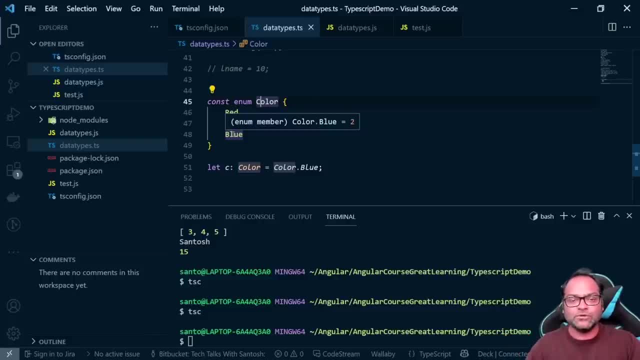 from this, but that doesn't need to be known. once your code is deployed on production, Just declare it as a const. that's it. So that's a very good use case And in case you want to trim down some bytes from your production bundle. 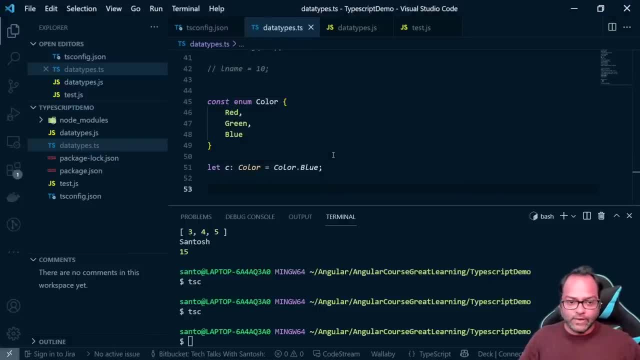 Tuples. tuples are. I mean, when I was using NET, I used to use it a lot. I mean, I think that when I was writing that NET code, it was really a new feature which was introduced in NET. 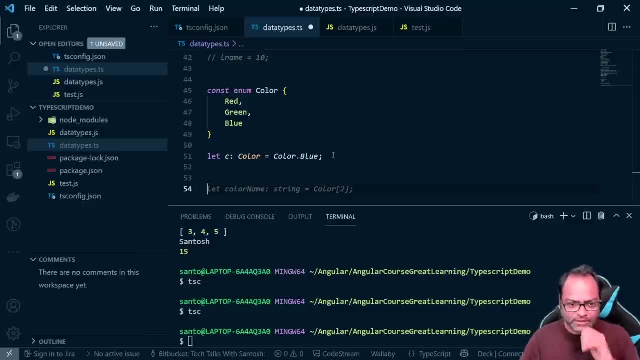 And it is there from long time in Python and very useful. So let's see, I mean what we can do is let's use tuples to swap two numbers, Let's see how many lines to code field, right, So I'll create, let swap numbers. 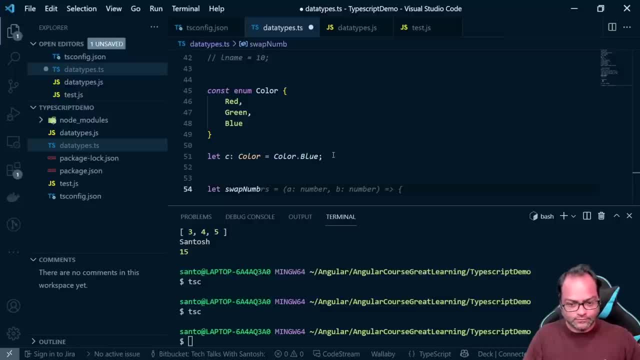 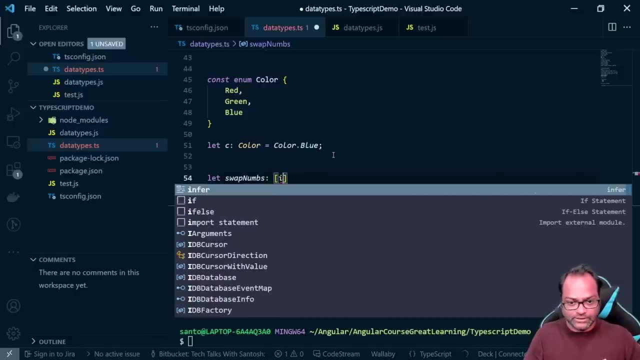 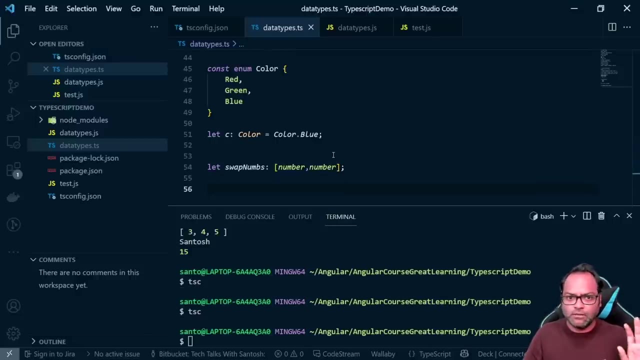 Which is type of integer- sorry, not integer. So this is type of number, common number. So this is my tuple and I'll write a function right now. So I'll say function, swap numbers. And what this swap numbers does is it takes two parameters. 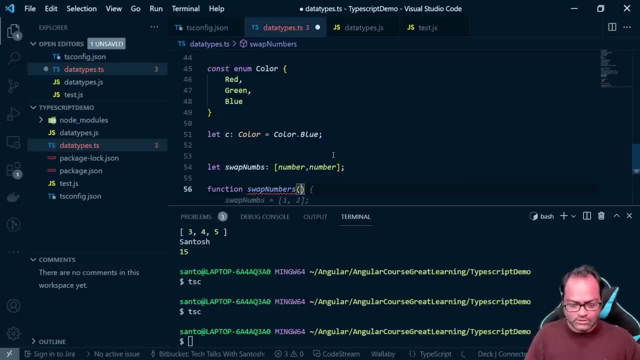 So I'll say it takes num one comma, num two, So these are two values it takes and it returns num two comma num one. Now let's use it. So what I'm going to do is I can say swap nums. 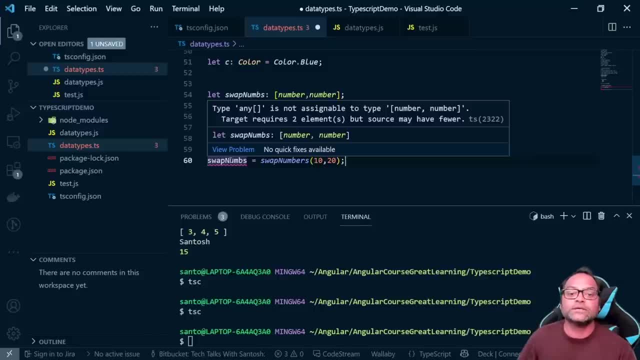 is equals to swap numbers 10 comma 20.. So let's see, it says: inning cannot be assigned. Okay, so here number. So here I have to just assign the return type as well. Now let's see what it returns. 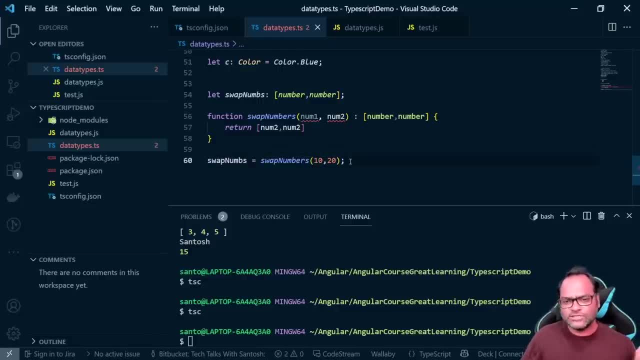 So it says okay, it returns number, comma number. And you must be wondering: this looks similar to arrays. What is the difference? So let me show you that. So here, if I try to access swap numbers of zero, this will give me a problem. 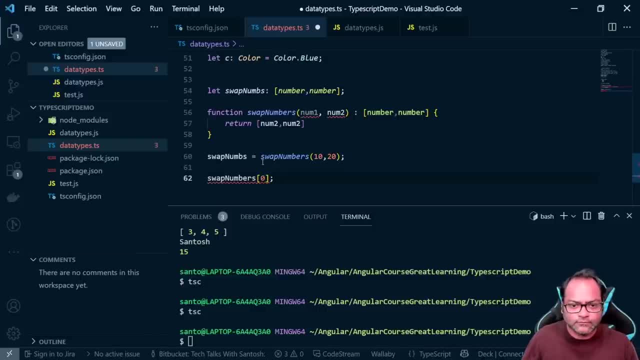 So you could see it's a little bit less than zero. So I'm going to change the variable name of the variable name to zero. And what this does is this: it gives me the variable name of the variable name And I can also change the variable name. 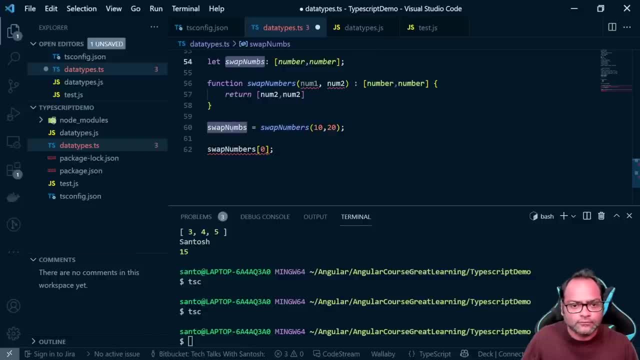 to zero if I want to. So so you can see, this is the problem. So let's go back and see. Let's say I'm gonna change our void And now my structure in the array is this tool: 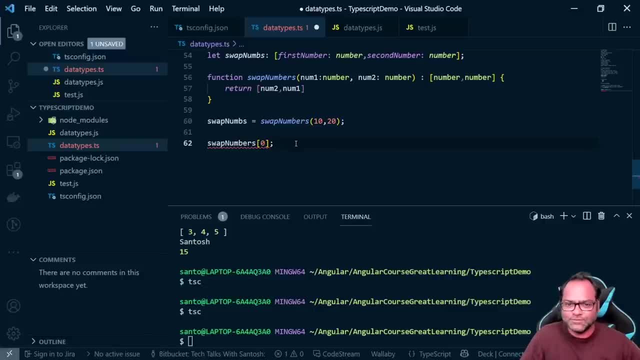 I'm gonna change the variable name to zero. So I'm gonna change the variable name to zero. So here you can see. I mean you must be wondering: okay, this looks similar to the Aries, But okay, what's the problem here? 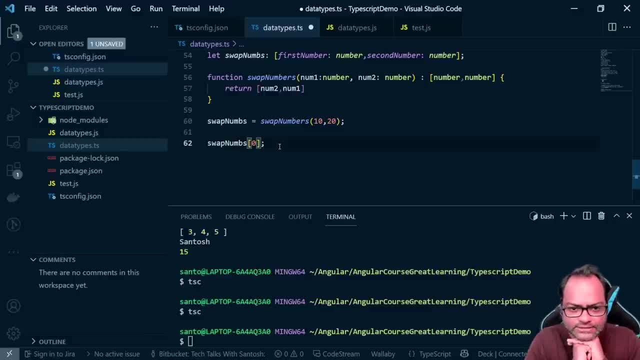 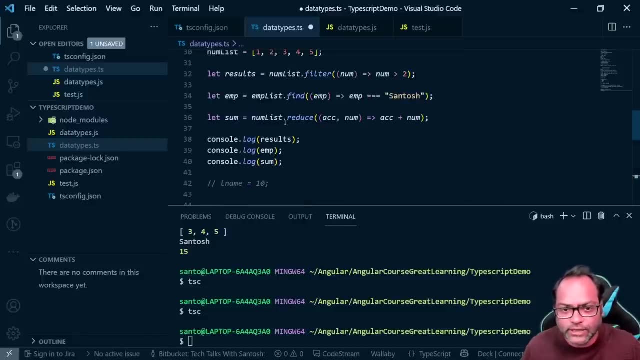 So you can see okay. So here you can see: okay, I can access this, swap numbers with zero. I mean, this is something which you can do with arrays as well. Here let's try to do that right. So for example, yeah, numList. 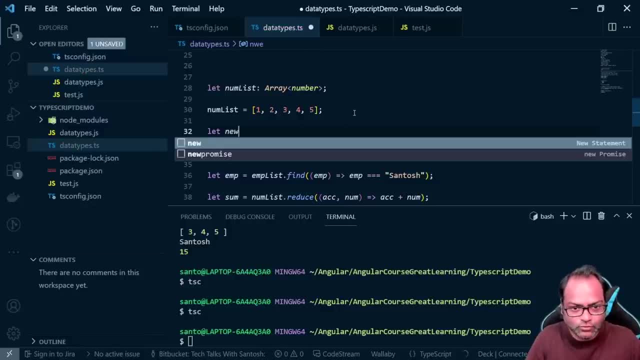 So I can say: let new num is equals to numList of zero. It works. So, if you know arrays index starts with zero. So zero one, two, three, four. So four is the maximum index which we can access. Let's try to enter five. 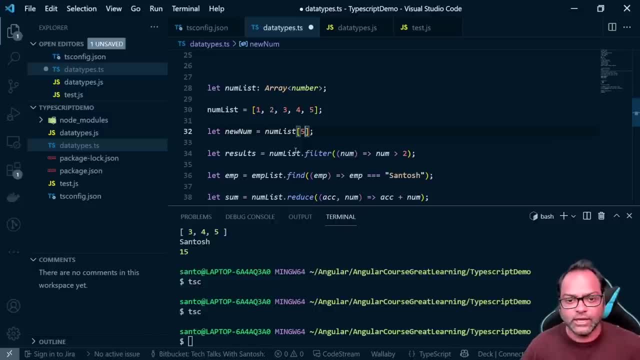 You don't get any issue here, I mean it's okay. The only problem will be once you compile your code. it will probably throw you an error, right, Because there is no element at fifth index. But let's But. 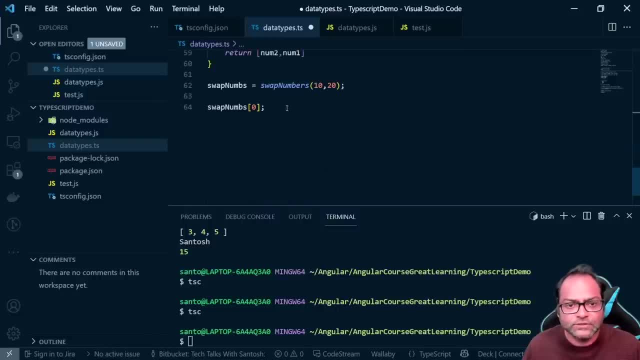 But. But let's try to do something similar here. So we have two numbers available inside this swap function, right? So you have first number and second number. So if I try to access swap numbers of two, Let's see Again. I just entered the wrong variable name. 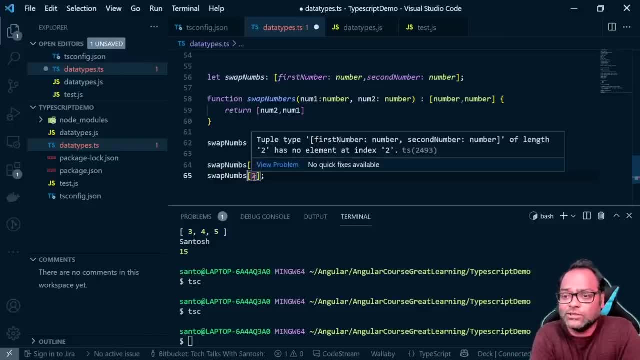 So here you can see. it says: this tuple has length of two, has no element at index two. Okay, If length two has no element at index two, So it is saying that this tuple only has two values. That's it. I cannot see any value at index two. 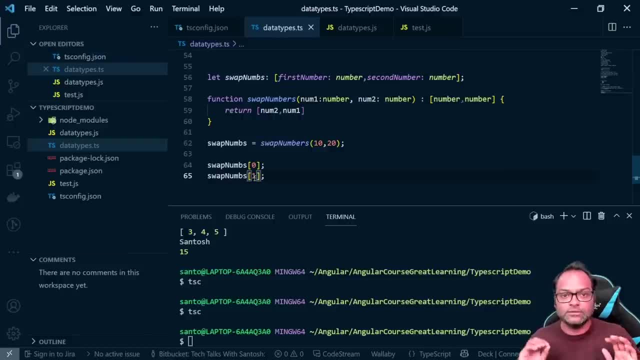 If I try to access the value at one, it will just give me the value, That's it. It will not give me any exception. So what do you think this tuples can be helpful at? So let's say you have an API call which gives you, let's say, employee list and department list as well. 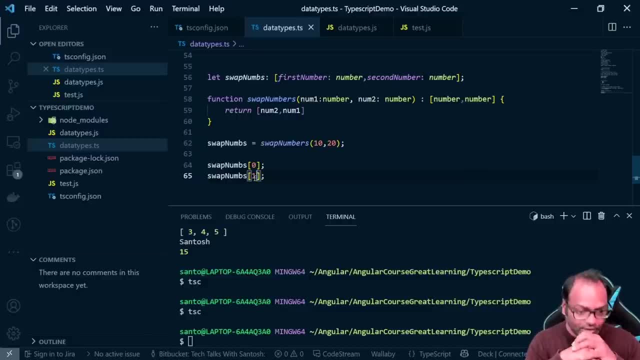 In most of the cases you can see that you have an API call. So in most of the cases, what you have to do is, of course, you have to go ahead and create two separate APIs, or probably you have to go ahead and find the objects and then you have to assign it to two different properties to return it from your function. 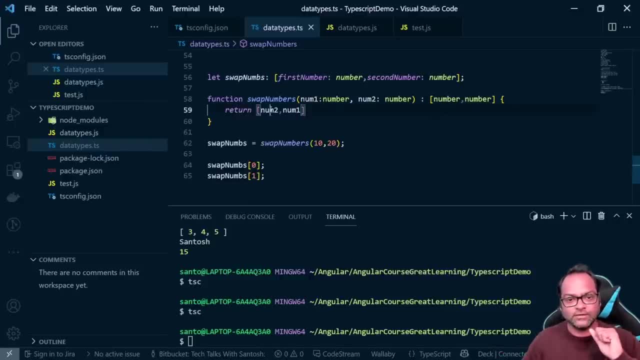 But using tuples you can actually easily do that right. You can just return first value and second value. So you can probably say: this is department and this is employee And your variable can be of type employee and type of department And it can just: 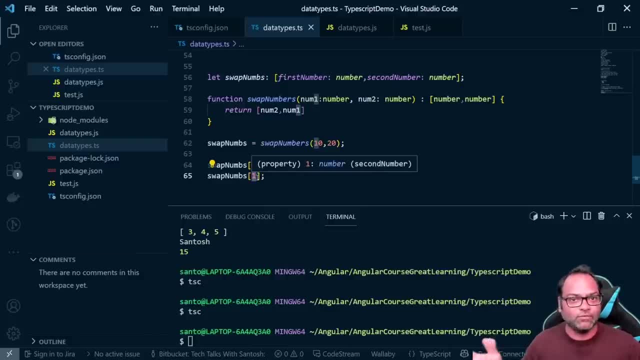 First the value by index, using zero or one, So you can say of employee or zero. or zero will be, let's say, employee and one will be your department. So that's what you can actually do using tuples. React has a lot of use cases for tuples. 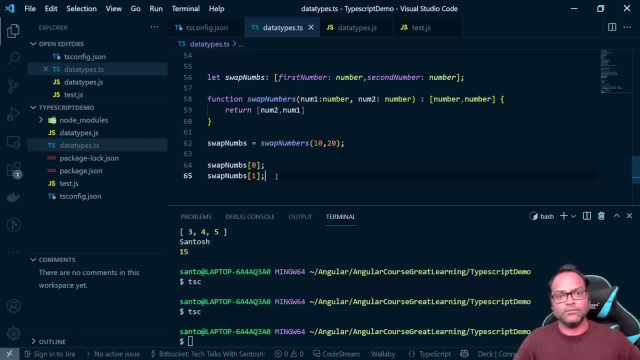 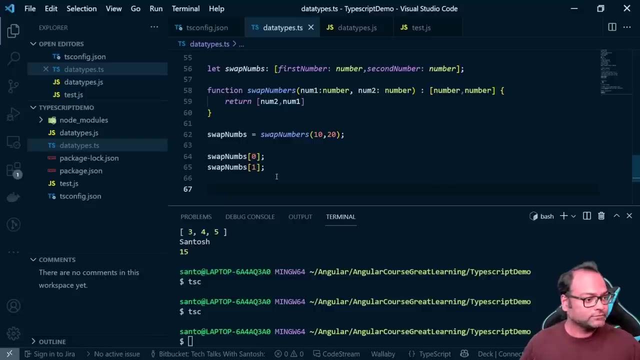 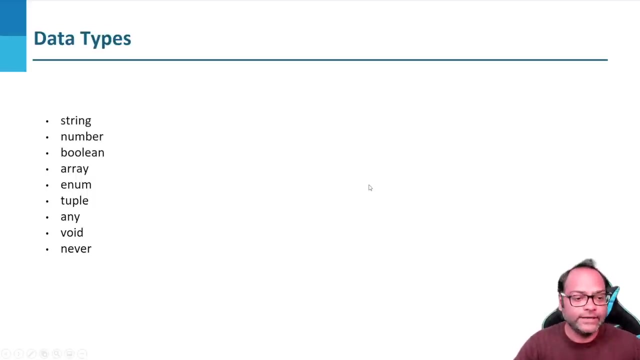 I have not seen that much use cases in Angular, but probably some advanced cases So, which I have never been across. But yeah, this tuples are really useful. in case you have a function which returns multiple values, You can use tuples. So let's see other data types. 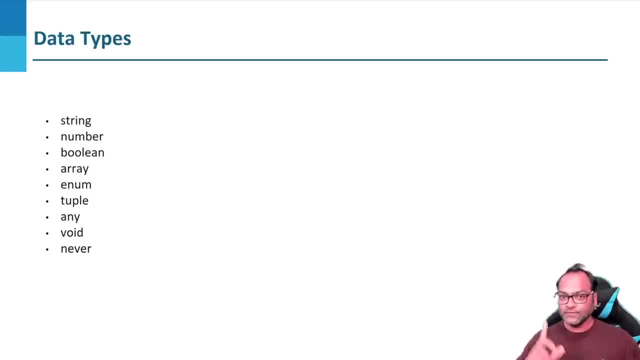 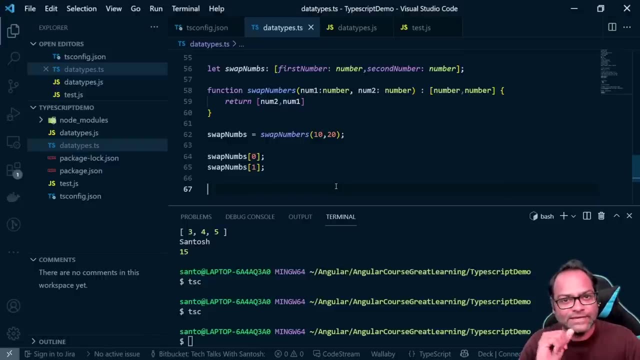 So now next data type which we have is any. We actually saw any data type. We actually saw any data type when we were going through arrays, remember. So any is kind of, let's say, in JavaScript, if you remember, in JavaScript you don't have any data types. 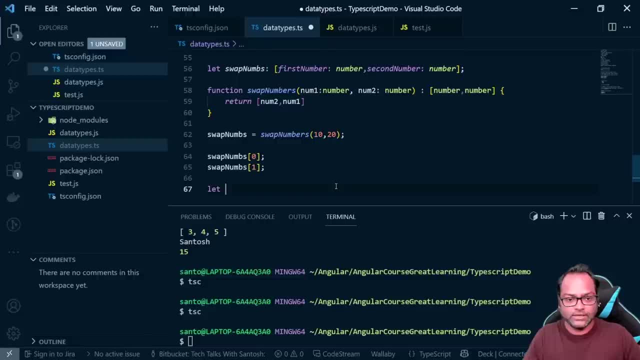 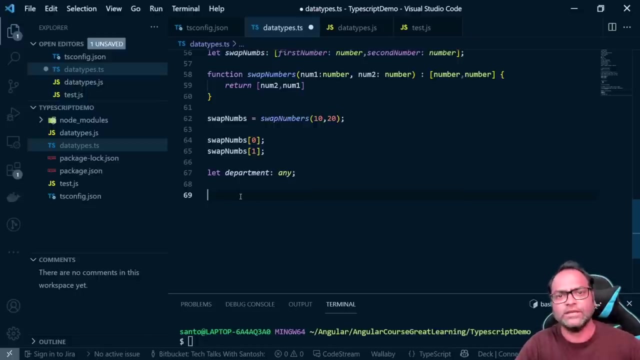 So any is kind of equivalent. So if I create a variable, I'll select department, which is type of any. So if I create a variable with type as any here- So I have department variable, which is type of any- I can assign any value to this particular variable. 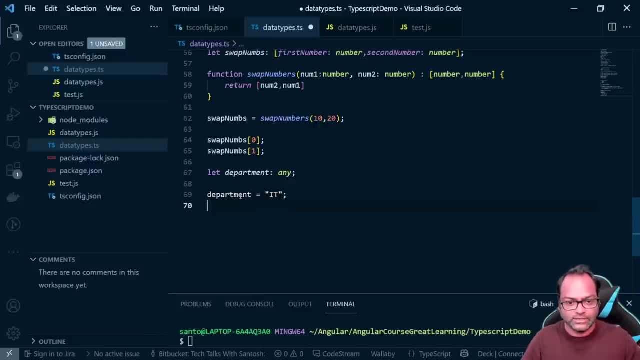 So I can say: department is equals to IT, Department Equals to 10. And it will accept it. It will not throw any exception. The first thing which you should do is do not use any in your code base. So try to avoid any in case you have an existing code base. 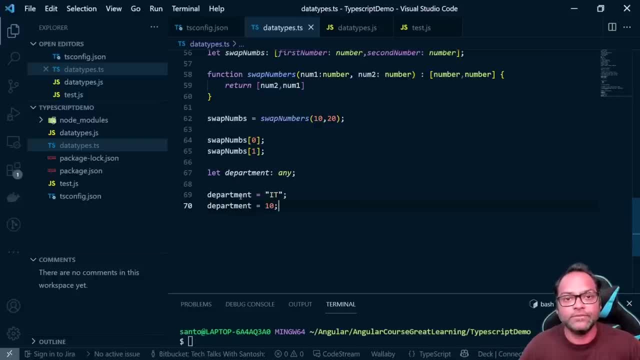 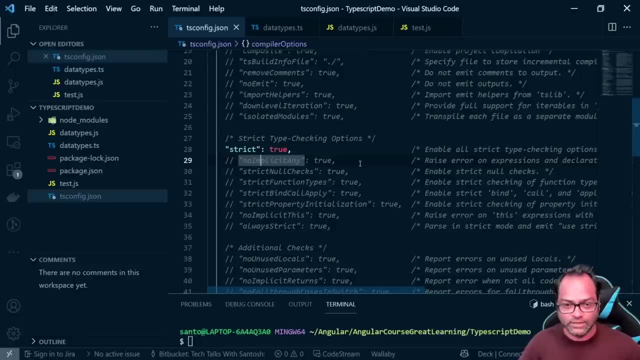 Try to move away from any and use the correct data types in case you can. Otherwise, there is something called implicit any droop flag, available here as well, which stops you from using any by default. So if I just enable this, let's see. 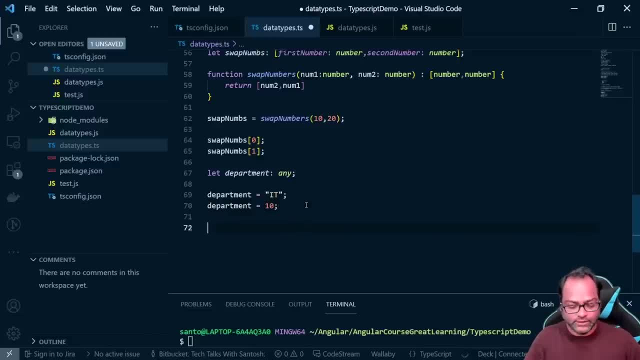 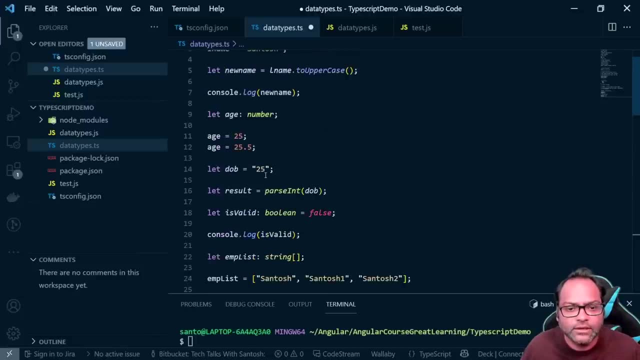 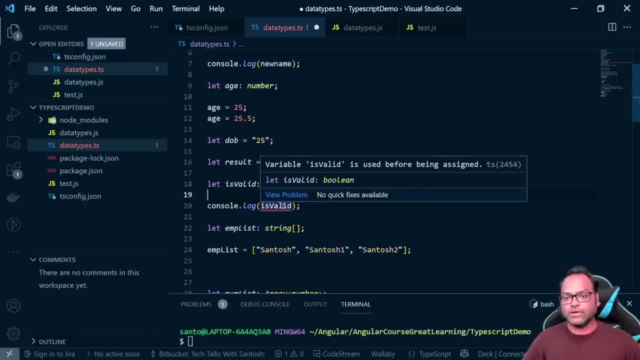 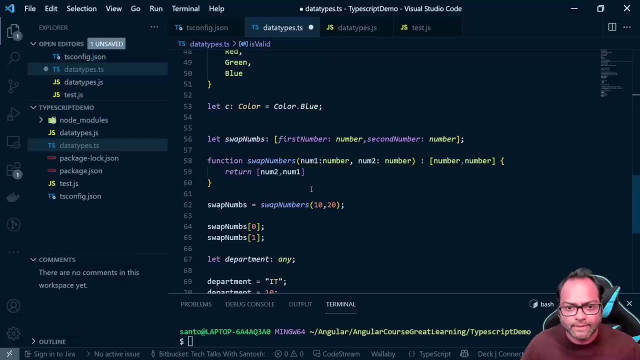 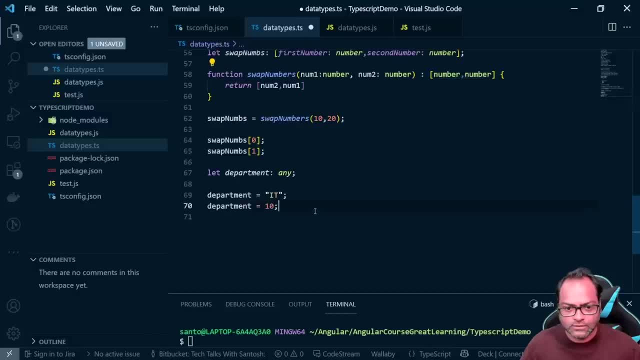 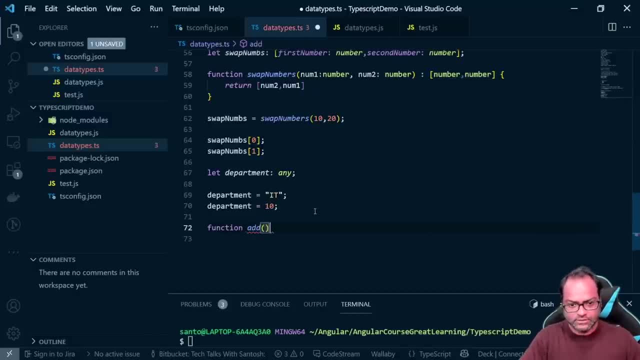 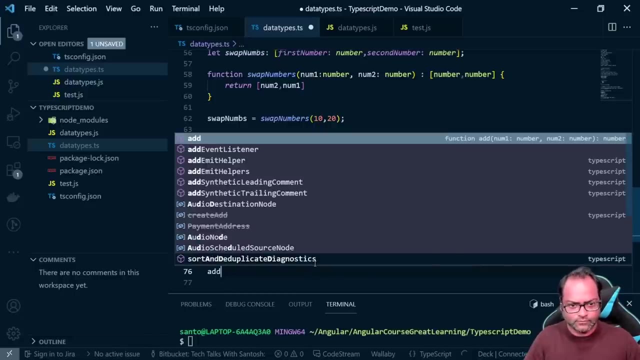 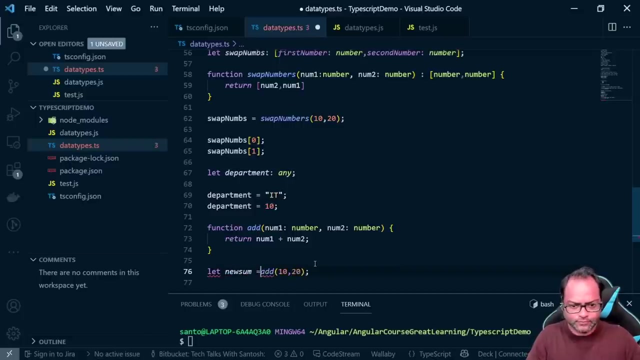 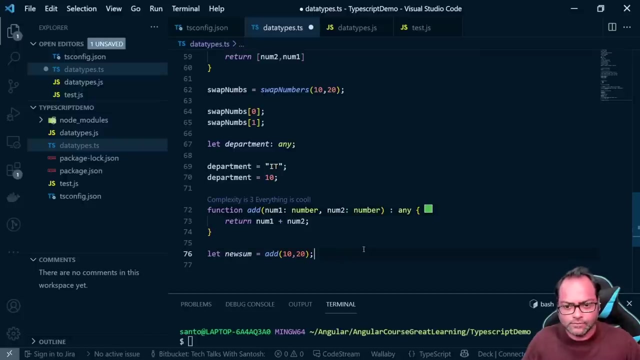 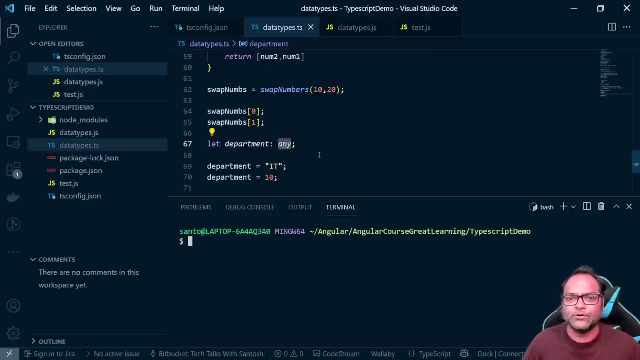 Let's start create a function, So it's a function ad. Let's start create a function And here we'll see implicit any, because we are. we are actually saying number, so it cannot give a similar. but yeah, and I don't try to use any, probably I'm not able to get the error because we are. 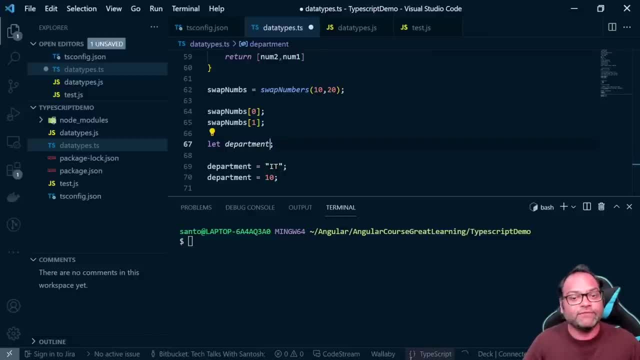 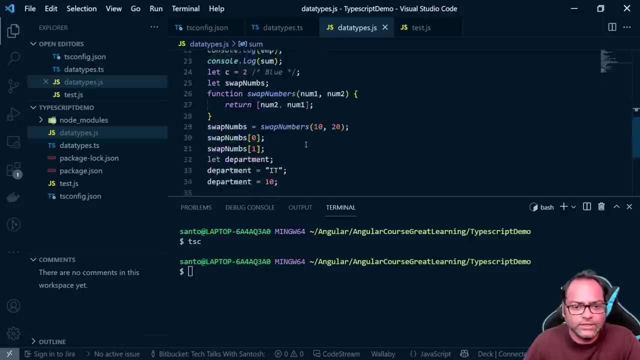 saying this is any, but even though if you don't give any right, so if you just create a variable without mentioning any data, you will also see that okay, this is also type of in. so let's try to compile this for TC and let's see the output right, so it will work. is a work as it is, I mean. 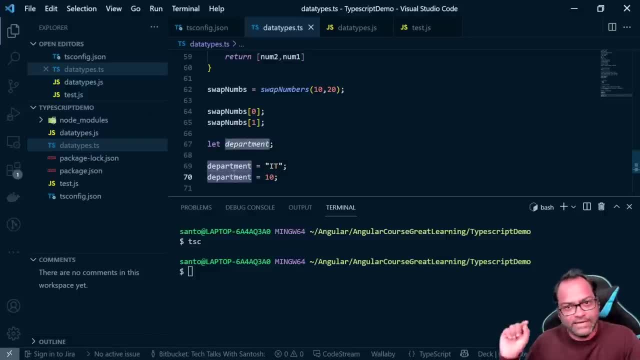 there is no real types assigned, so you don't have any type check and your application or your code may fail in production, right, because you are not using the time safety feature. so first thing which you should do is not do not use type any anywhere, in case you have an existing. 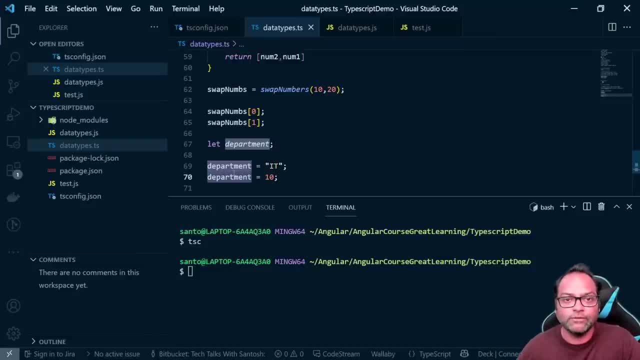 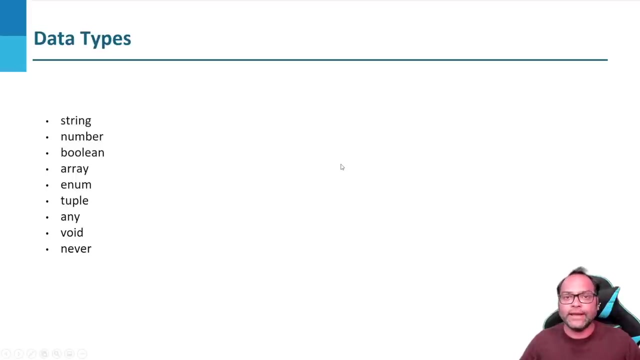 code base, try to actually incrementally do it. I mean you, of course. if you have a large code base, you cannot do it at once. you can do it slowly, slowly, in iterations. that's what you should target about. so this is any. and now the other data types which we have. we have void and never 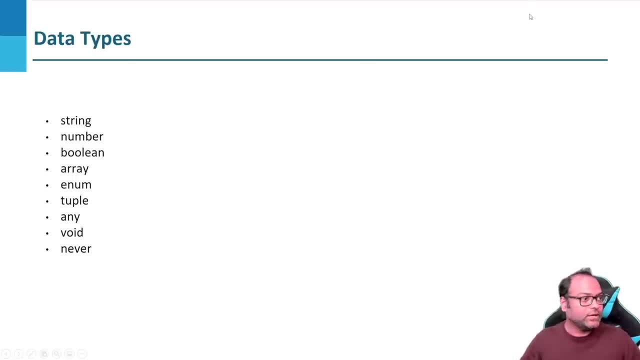 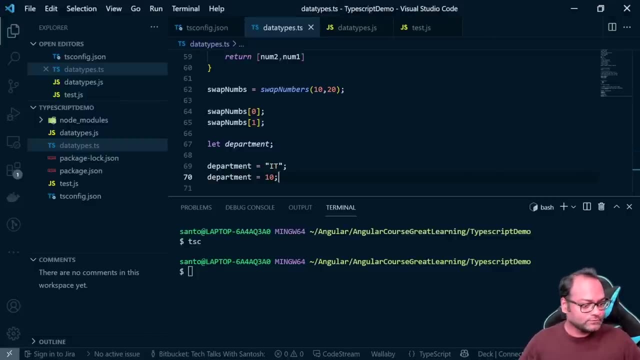 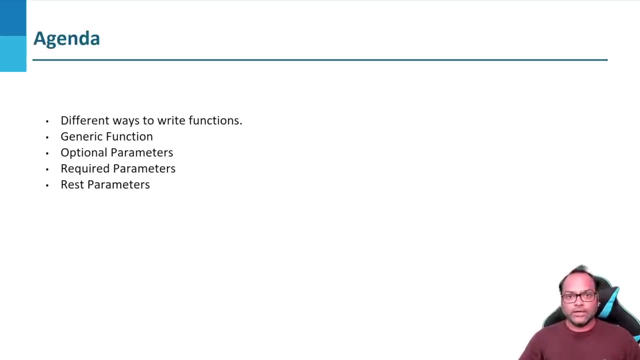 so let's go ahead and see. but before that, I mean before discussing about these two types, we will go through functions. so, uh, in functions, uh, functions are what, like some, some uh set of instructions which you write. uh, for example, let's say, if I want to add two numbers, what I can do is I can write a function. 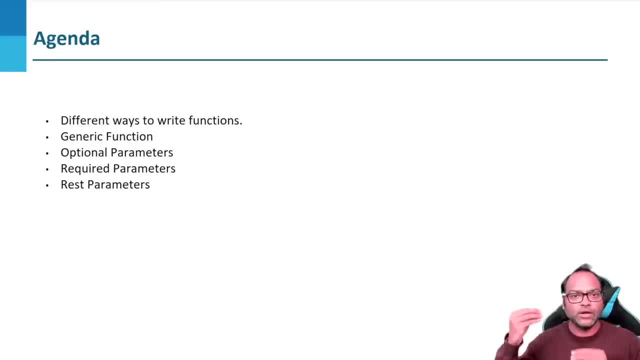 which will have the instructions on getting the input, how to add those functions and then return it. it's kind of, uh, probably a reusable thing which you can actually go ahead and reuse wherever you want- or it can be your business logic as well- right, so probably getting the API data that can. 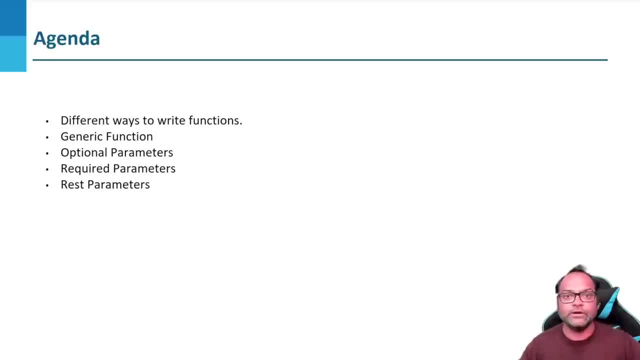 be a function. so, uh, in this particular video we are going to talk about different ways to write functions. so we'll talk about how you can write your function in typescript. then we will talk about generic function. we'll talk about optional parameter, required parameter and rest parameter. 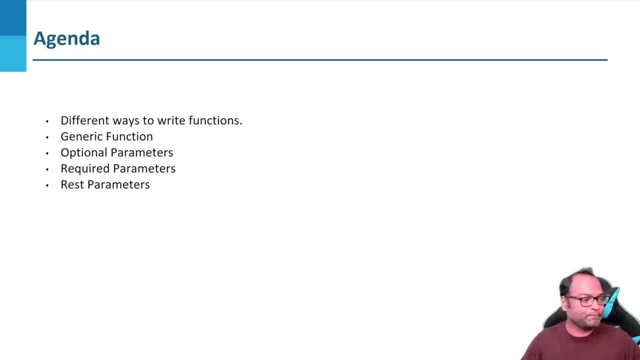 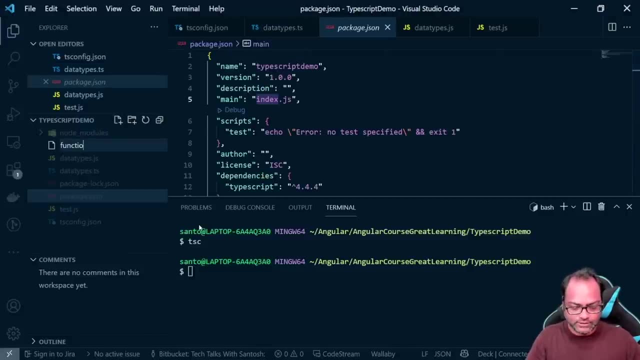 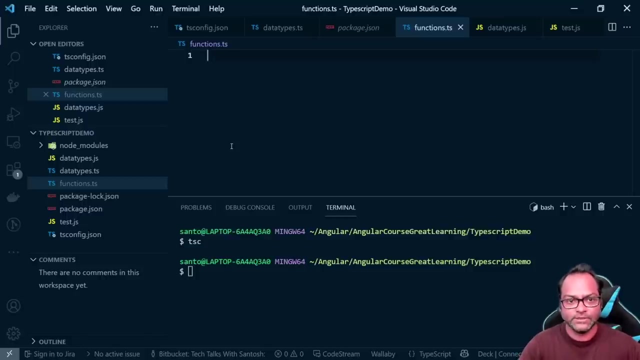 so let's, let's go ahead and do that. I'll create a new file for functions. I'll call it as functions dot these. so first let's talk about the ways in which you can write a function in typescript. there are multiple ways. the first first is of course name function. for example, I can say function and then function keyword and. 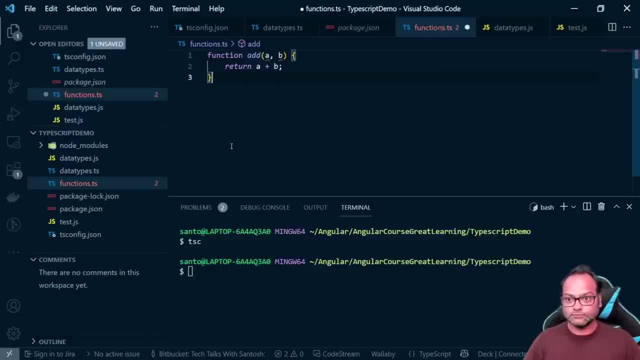 then I can say add, and this is functions. dot d is right. yeah, so you have add functions and now you have two parameters and it returns a plus b. this is generally what we write in JavaScript, right, but in typescript, as we said, we will be using type safety, so I can remove this and I'll 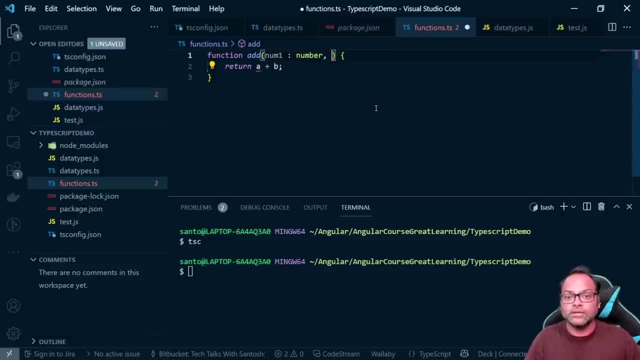 say: this is number one which is type of number, so I'll be mentioning the type of parameters which it can accept. so I'll say, okay, this is number which is type of number and this is actually, as I said, this is GitHub copilot which which is being used here, and then I can return num one plus. 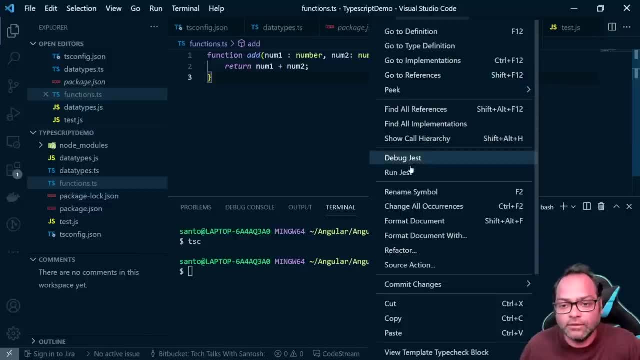 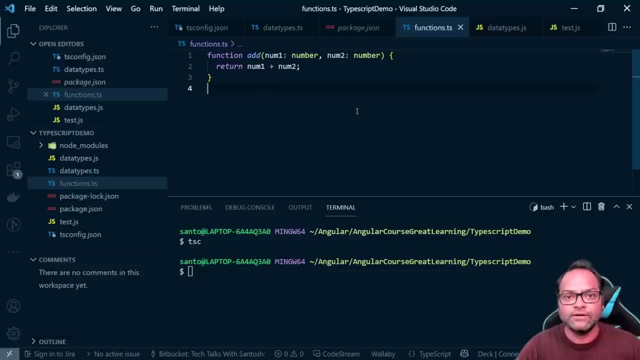 num two. so in typescript you always have type safe functions. so uh in, if you, if I have to actually add a function in Java, if I have to create a JavaScript function for ad and I don't define any uh types right- generally I don't- then I can accept strings as well and it can break your code as well. but 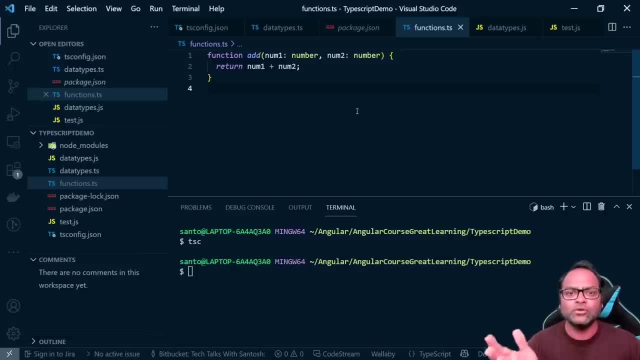 here we are saying: okay, this function, this ad function, is going to be a function which is going function can only add two numbers, so that's it. that's second care of, and due to inference, due to inference, this ad function knows the written type as well. but I will suggest always have the 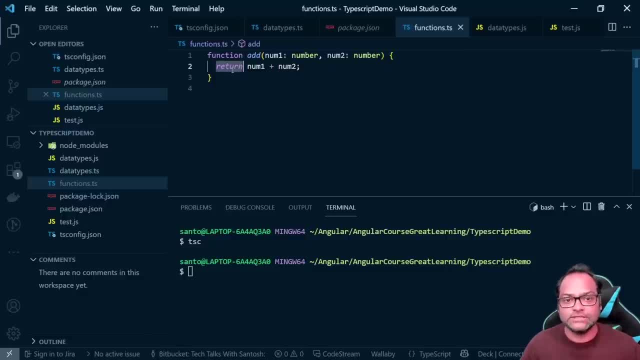 written type. let me tell you the reason why. of course, one reason is for compiler and what in case? you try to add two numbers but you miss the written keyword, which happens a lot of time. I mean, of course, it happens with me, uh, sometime. I just miss the written keyword and I just keep thinking. 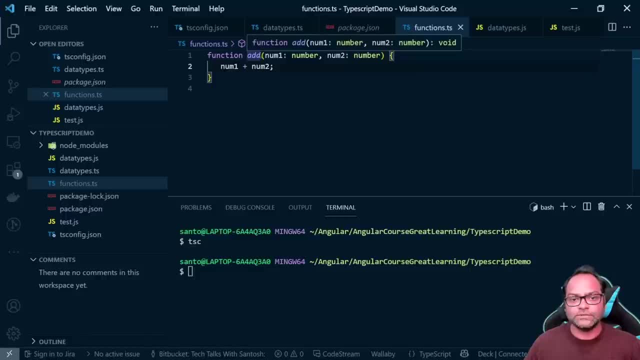 why this function doesn't return anything. let's see the written type. so it says it's void. remember the written type void, which we spoke about or saw in the previous slide. so void it means it will void. it means it will not return anything, right? so this function will not return anything. just to make sure that, okay. uh, you don't. 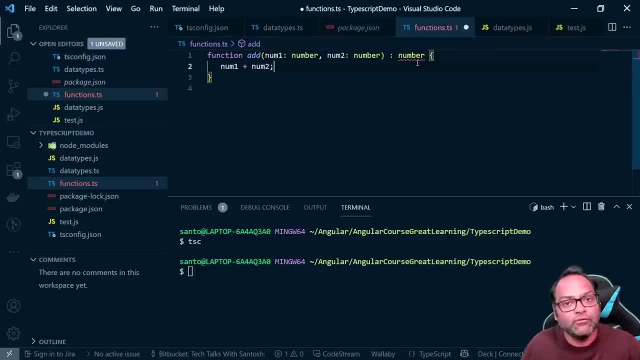 get into such issues. if I define the return type now, you will start getting an error. so it will say: okay, the function whose declared type is neither void or any must return a value. because we are saying that this should return a number, then we have to put in a return number. 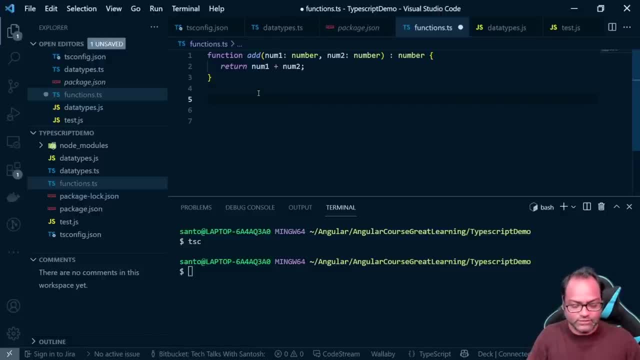 that's. this is this is your first way to write function, and then you can say: okay, let, or let's do consolelog. add 2 comma 3, right, so I can just run tsc to compile the files. and then you can use node functions and you will get the output as five. 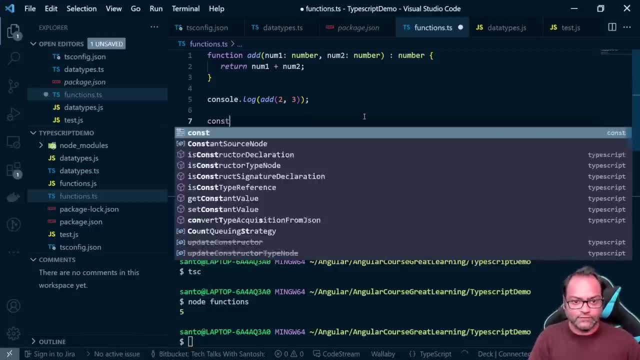 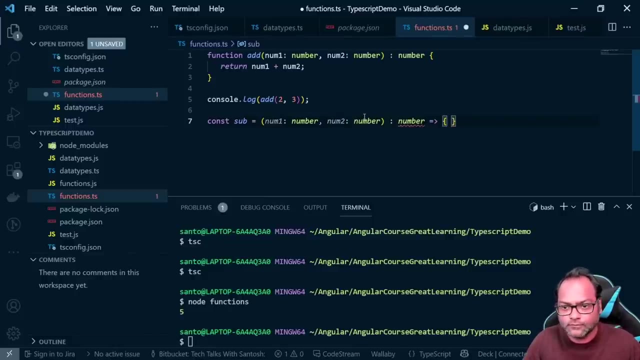 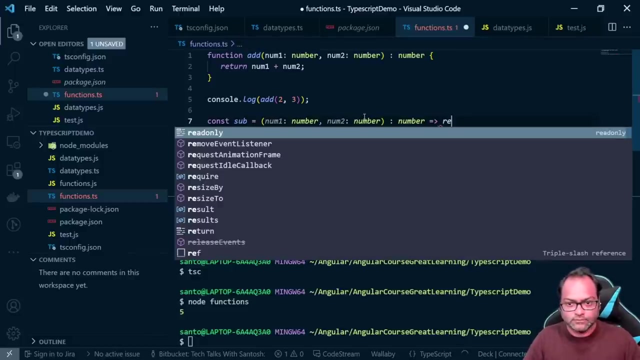 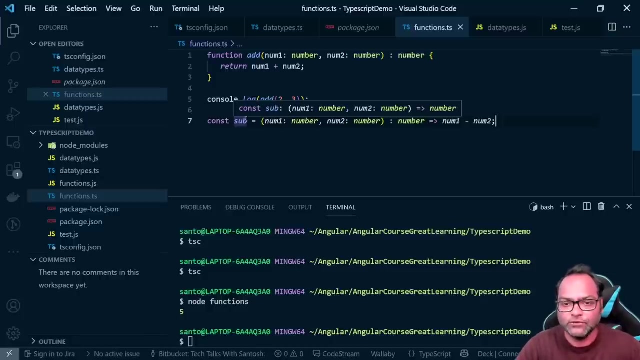 let's see another way to write a function. so you can also write a function like I'll just use: subtract is equals to, or remove this, uh, this, um, and I'll say return, or you don't have to return. so this is also another way to write function. you can see: uh, the same right. so you have just you. 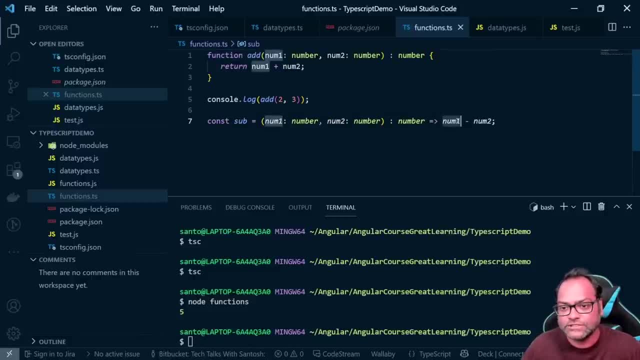 don't have function keyboard, that's it. so here we are saying: this is something which we know as a row function, right, so you have arrow function, I believe used here. and then you are saying: the sub function takes two parameters, number one and number two, and returns the number. and uh. within this it will say number one minus number two. so this is another way and let's try as a host, which is called intализär. Number1 is much more different in the programming structure. actually, I'm not that specific, but I'm gonna. 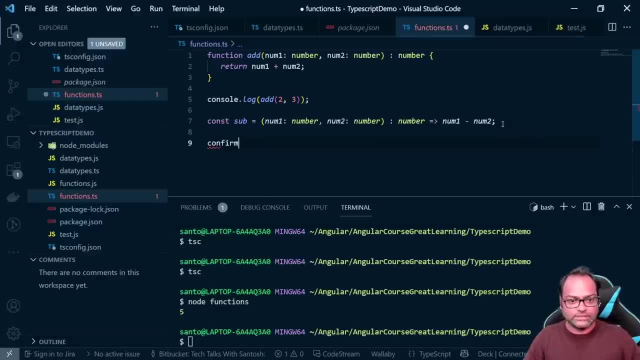 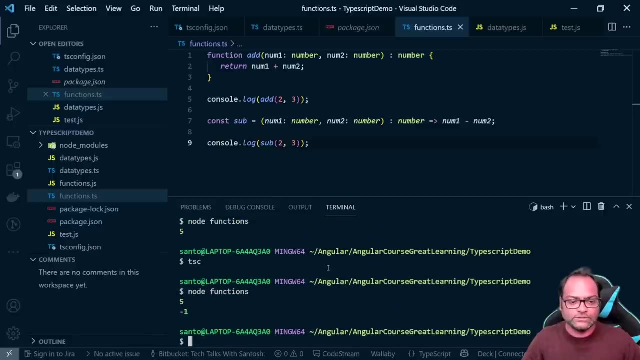 going to use in a few examples, says so, let's say, and then Error brig, then what will it take? and let's try this out and see: subtract two minus three, of course, which will, which should return minus one. so let's see: run dsc and then known functions, and we have minus one as output. 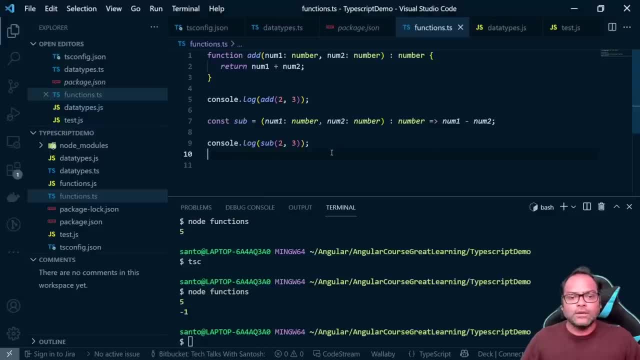 there is one more variation to write a function. let's use constant multiply and rather than using arrow function you. what you can do is you can actually use a function keyword here and then you can say return number and here you can say: okay, oh sorry, you don't have to use arrow function. 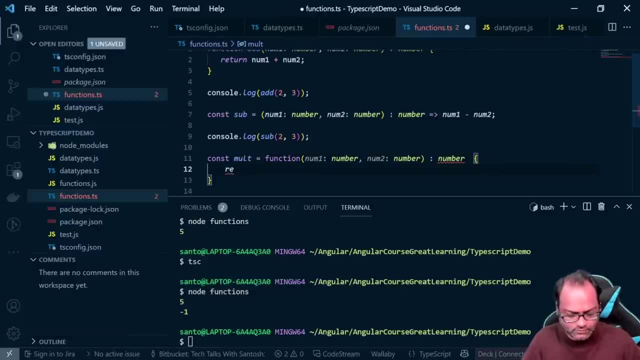 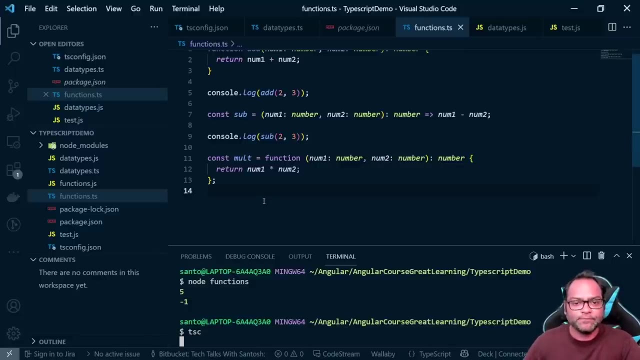 now you can say return number into. you can say return number into. so this is another variation, the way of writing a function you can use. i mean whatever type you want to let's see the output right. so if you run tsc, let's go to functionsjs so you can see. 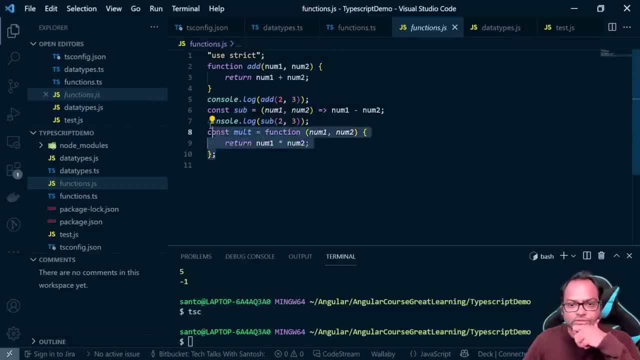 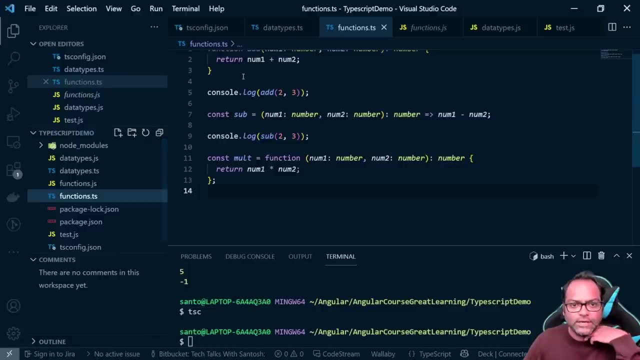 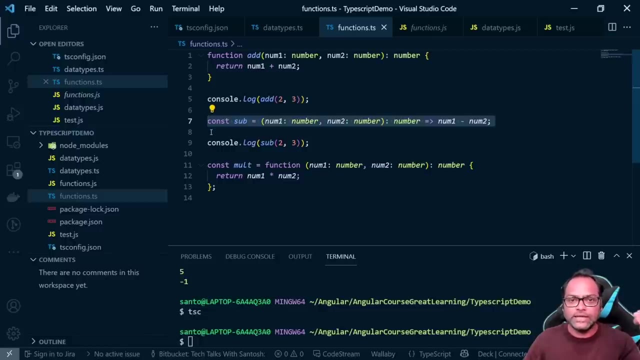 this is your subtraction, this is a multiplication, so all the types are stripped and this is your normal name function. so this is name and this is a named function, this is a function expression and this is arrow function. so this is, uh, three types in which you can write a function. 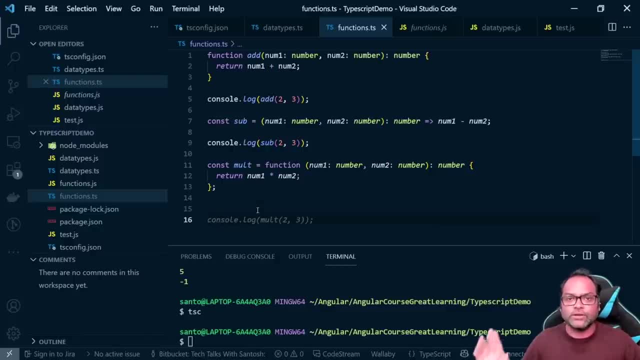 and there is more to it, but you don't have to worry about it, you know this is. this is the minimum information which we need to start working on our angular code base now. after this, let's see some example of optional parameters, required parameters and rest parameters. so let's say: 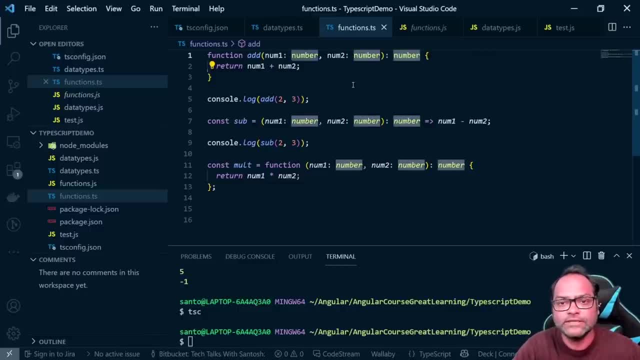 now you have this add function. but what you need is you need to write a function and you need to add three numbers. but third number should be optional. so how you can do that? so here in type script you can say number three and you can put a question mark and say type of number. so now you 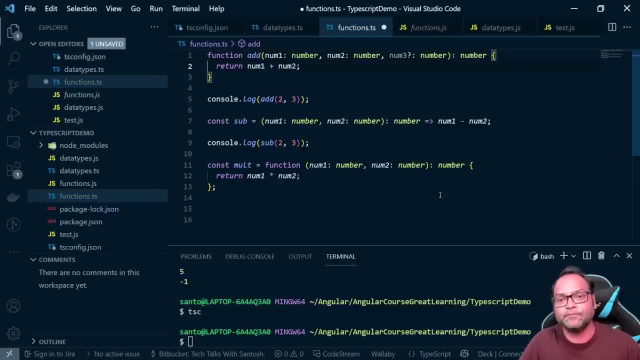 can see, num3 is optional and your add function still works. if i remove this, you will start getting an error, because this add function requires three argument. we have just passed out the add function and the add function requires three arguments. we have just passed two. so this is this is known as required- sorry, optional parameters. so i can use. 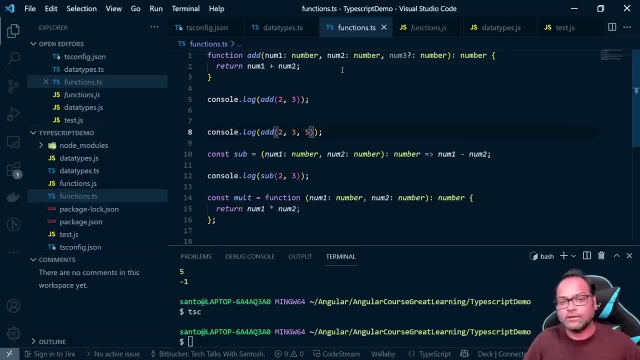 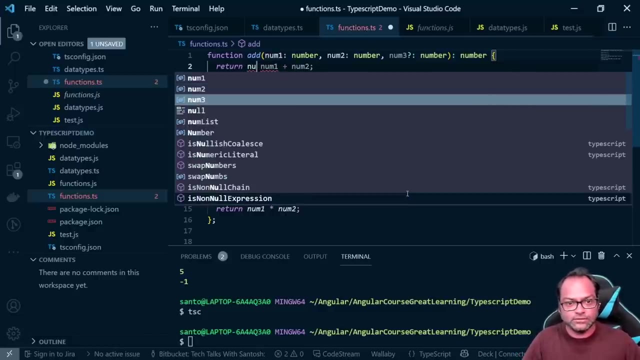 it with two values and three values as well. but i mean you must be wondering how about here? right, so how to use it here? uh, i'm just adding num1 plus num2. you can use, uh, the optional chaining here, so i can say num3 if num3 exists, so i will say num. 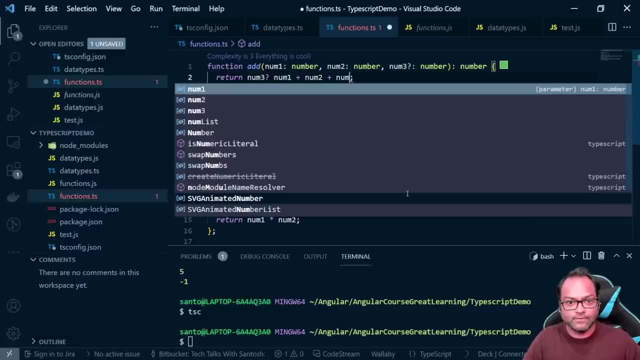 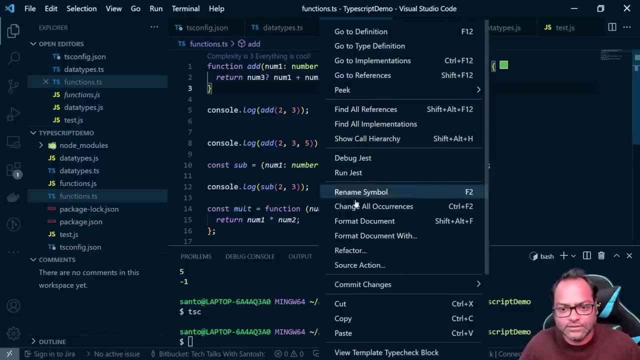 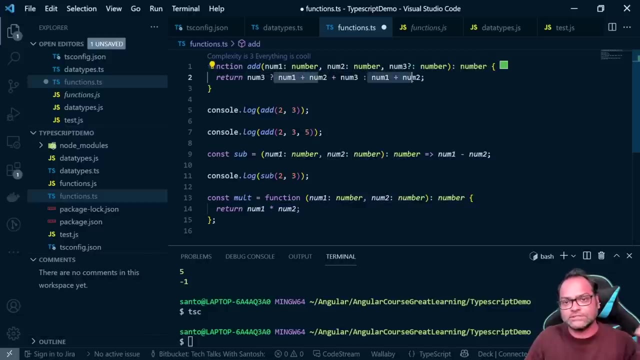 1 plus num2 plus num3, else num1 plus num2. so this is uh, if else statement in a single line. so here you can see. so it says: if num3 exists, num, add three numbers, if otherwise, just add two numbers. uh, this is not optional chaining. i'll talk about optional chaining, chaining in probably. 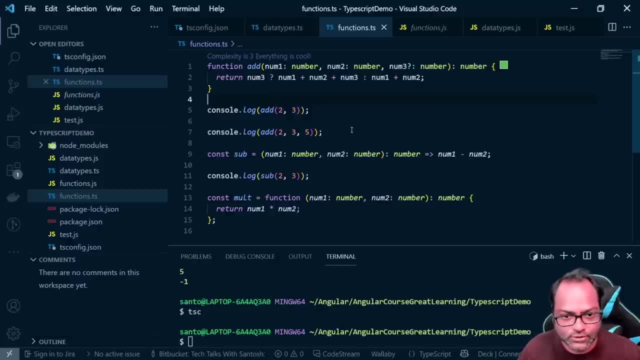 in next videos, in upcoming videos. this is not optional channel, sorry, sorry for that here, uh, you can also use. so, as i said, this is optional parameter. there is something called require parameter as well. so here let's say, i need three numbers, but third number is required. so 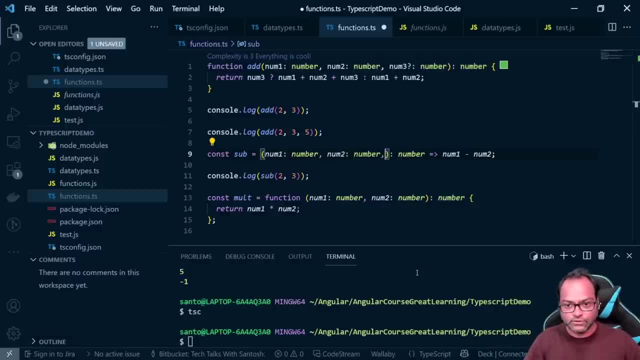 i mean you can still go ahead and avoid that. so i can create third parameter, num3, and i can assign it a default value. so if no one passes this value, 10 will be used. so i can say num1 minus one, uh, minus num3, right, so num3 has like default value of 10. 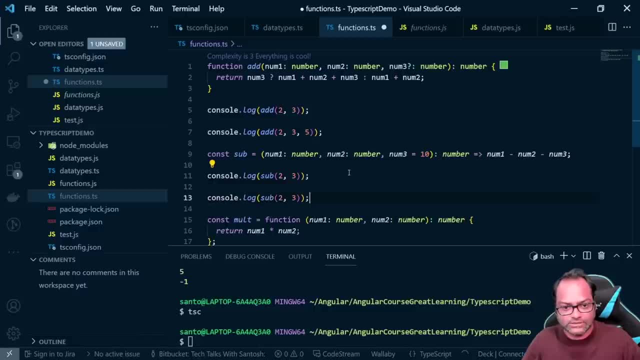 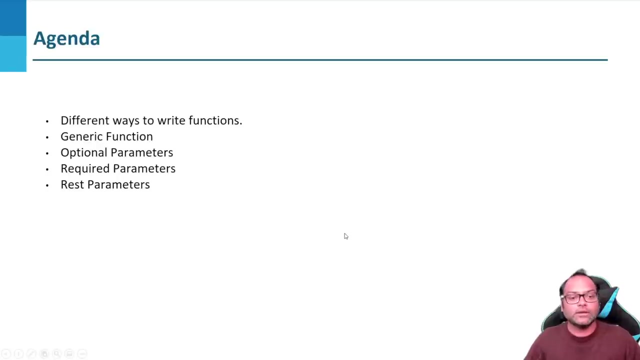 if no one passes, then will be used, but in case i pass the third value, this value will be used. so this is required, and so this one is required parameter and this is sorry. this one is optional parameter and this one is your required fact. so we also have something known as rest parameters. what is that? let's? let's go ahead and see that. 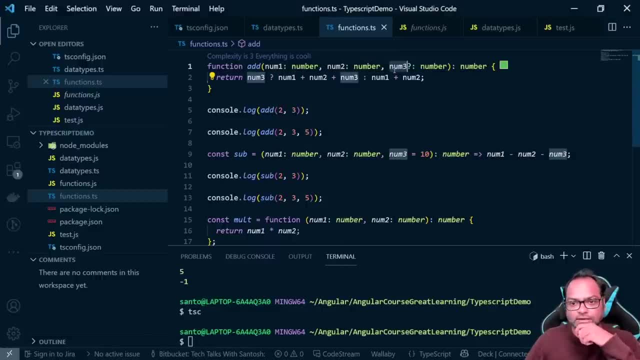 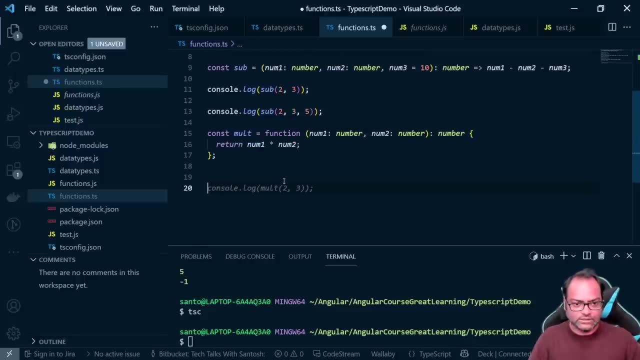 so now, uh, this function has required a requirement that, okay, third parameter can be optional, and this is where it is required. but let's write a function. so let's say, uh, function and two. okay, i'll just start, i'll say: add two. and here the thing is, i can pass n number of arrays and number of values after this. 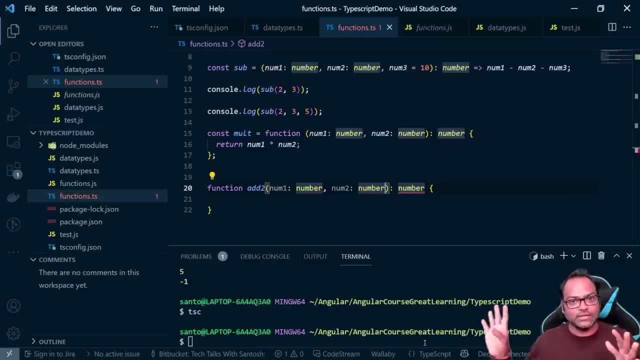 so i have two numbers, but after that i can just pass the n number of arrays. that's the requirement. how you can do that? so i can say num3, which is number array. so i'm saying: uh, this you can see, i mean. so, thanks to go, github, copilot, it is writing code for me now. 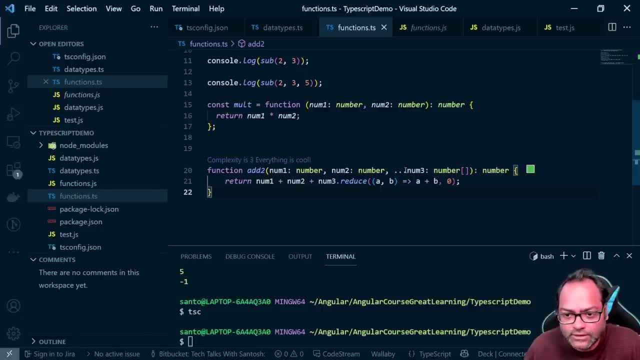 so here you must be wondering what is happening here. so here the third parameter is array. so i'm using reduce to make sure that it come, it actually sums everything and then adds in number one and number two. let's see how to use it. so i can say console, dot log. so i can say comma two, comma three. 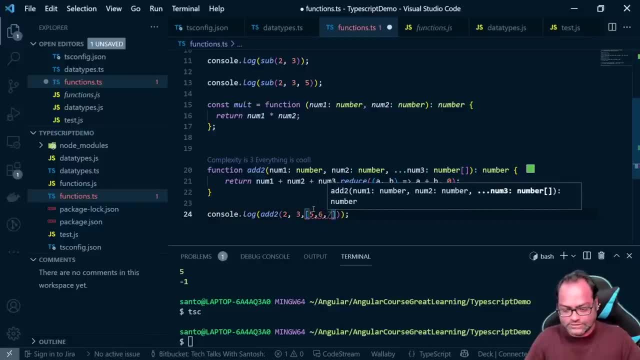 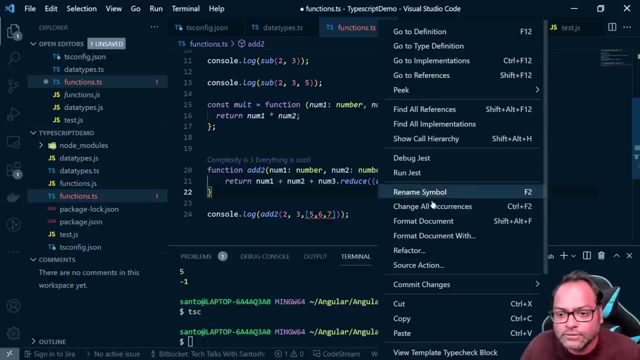 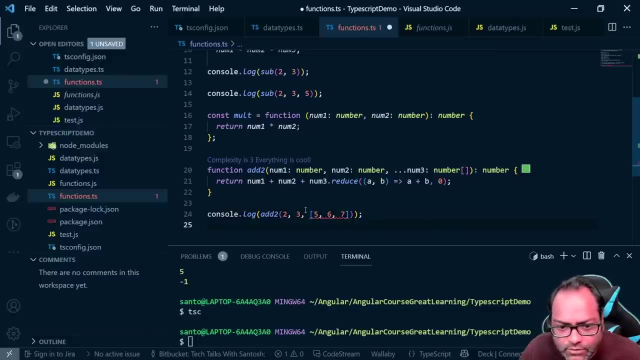 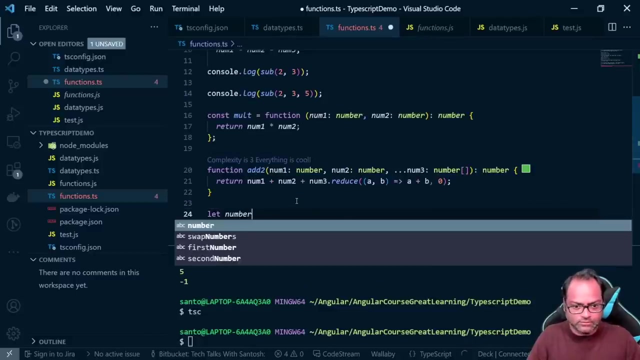 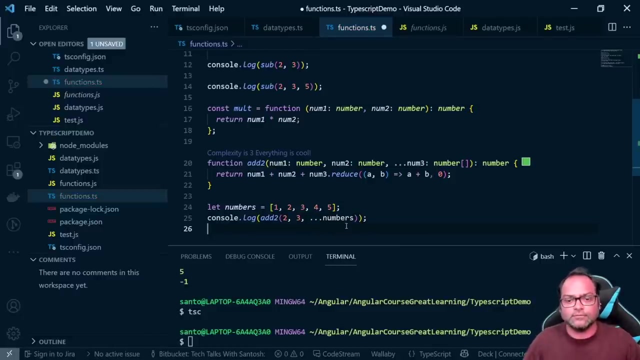 but i can also do five, six, seven, right? ah, argument of type number is not assigned to type. okay, let numbers is equals to variable. here should be okay. yeah, so we are using this rest operator, right? so I have to pass, like this, rest of numbers. so here it will be 2, 3, 2 plus 3 and 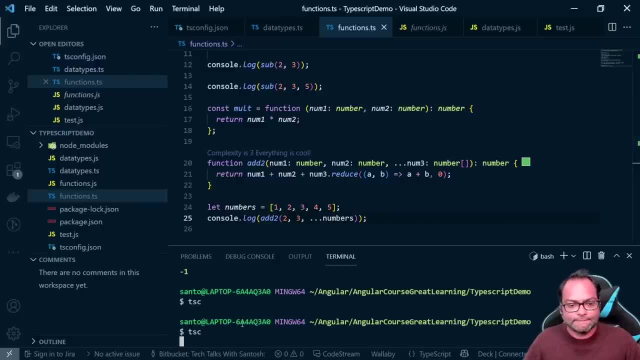 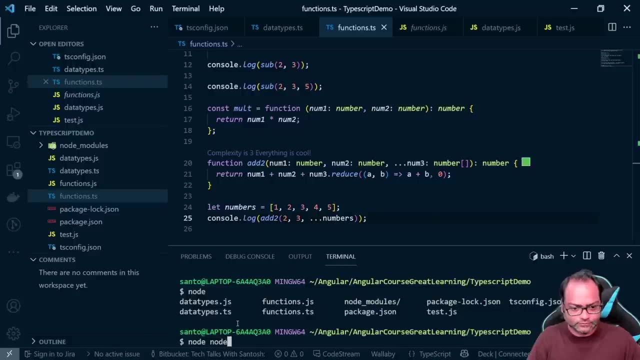 whatever the sum of this number is, let's see DAC and then we can see a node and yeah, so it comes to 20. so this is how you can use the rest parameters. so in case you want to pass n number of numbers after this, you can do that. I mean in previous thing and previous. 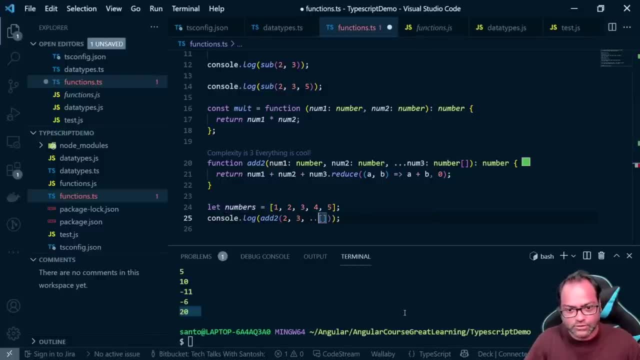 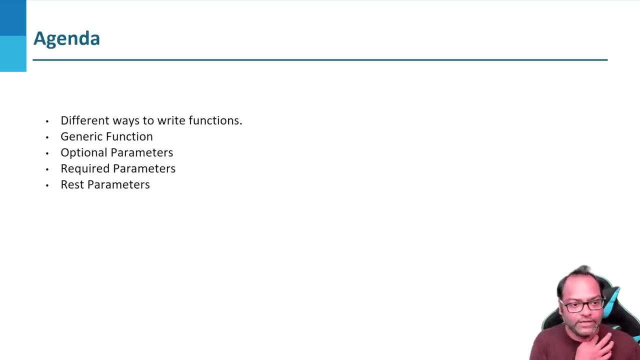 without doing this. you can also do this, but you have to say dot, dot, dot, and 5, 6, 7, and I mean you can go as much as you want, right? so this is how you can actually pass this: rest parameters or the rest values. so these are three, uh ways how you can actually play with the parameters, make 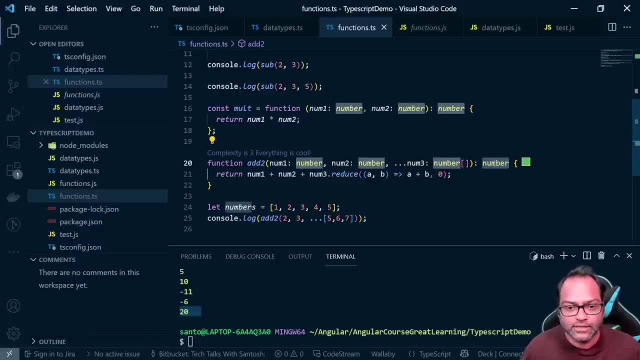 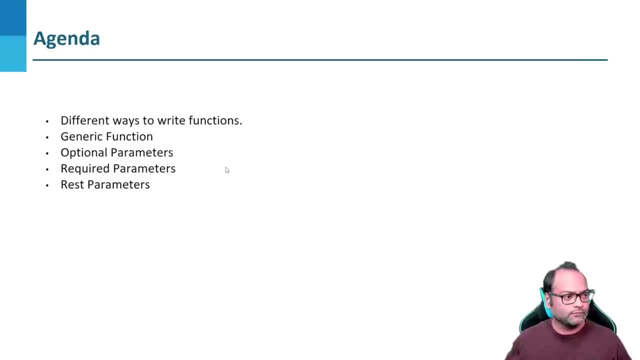 sure that you always, uh, define the written type and always define the parameters type as well. we will talk about generic function as well. if you remember, in previous video we saw and different variation of arrays. remember array and then angle brackets, and then we can different variation of arrays. remember array and then angle brackets, and then we can different. 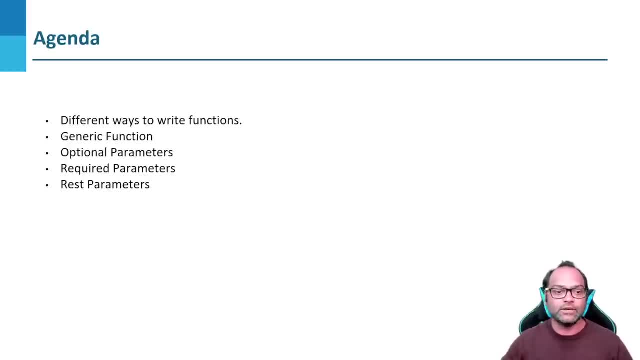 define what data type it will have: area of saying or f number. so generic functions are like. it can be like a function which can have like return type based on what you pass, so it will. it will be like it will act like a placeholder, so whatever you pass will be removed and uh will be returned. 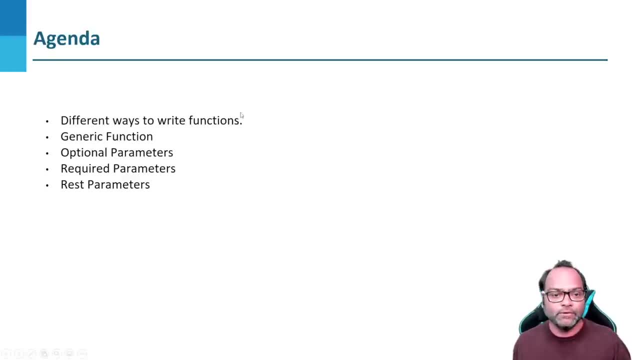 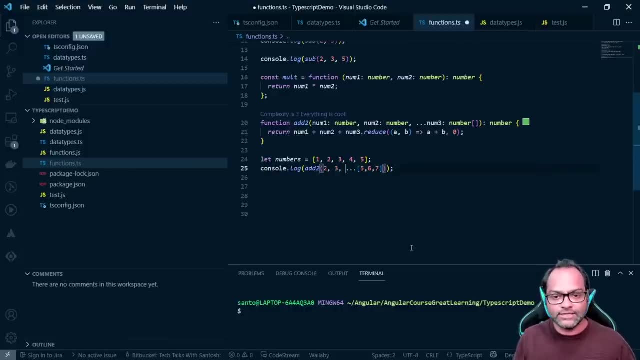 at the runtime. so let's go ahead and see that. but before before going to that, let me show you one more way to pass the data here. before going to that, let me show you one more way to pass the data here. before going to that, let me show you one more way to pass the data here. in the rest parameters we saw 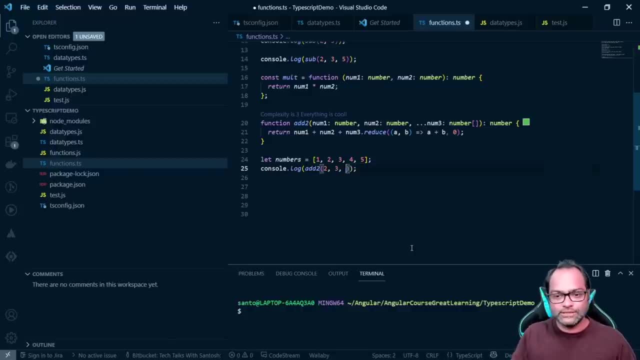 in the rest parameters we saw you can actually pass three dots, but you can also do this. you can just say five comma six comma, seven comma eight, I mean. so the way it works is the rest parameters. it will take these two as first and second parameter and rest of the values will be passed. 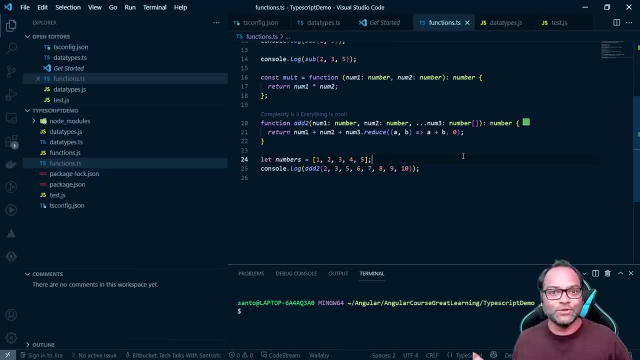 here number three, which is really cool, about rest parameters: right, so you don't have to go ahead and define 10 parameters or, uh, define 10 different parameters to actually hold those values. now let's go ahead and create our first uh, generic function. so what we will create, so what we can do is let's create a function which 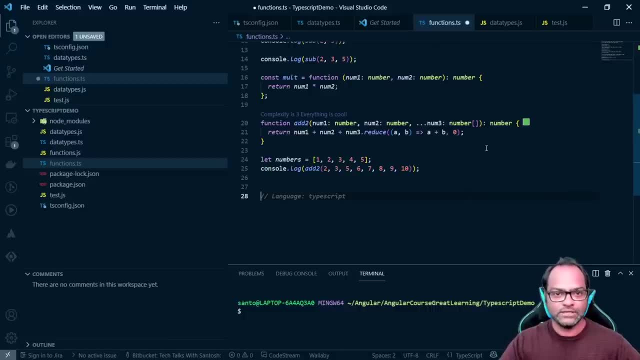 will take the array of string or array of number and then it can concate all the values and give it to you as a new array. let's see, let's see how we can build it. so here is the function. so it- uh, function name is get items. so we are saying this: T is our. 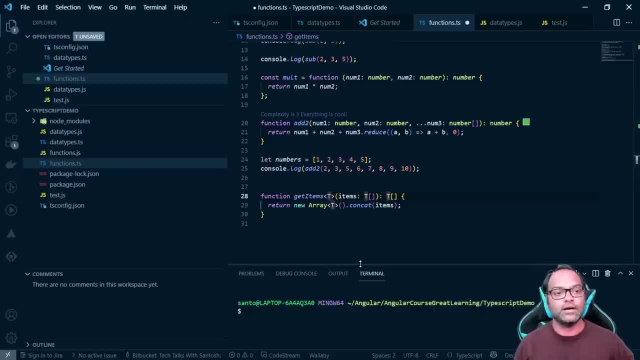 placeholder, you can call it any thing you want. so generally, uh, this was very confusing. when I started learning generics, I used to think T, some T means something, because everywhere, everywhere you go, you will find T, or every programming language you go for generics, you will find T. so it's not like that. you can also make it type and then just change everywhere from. 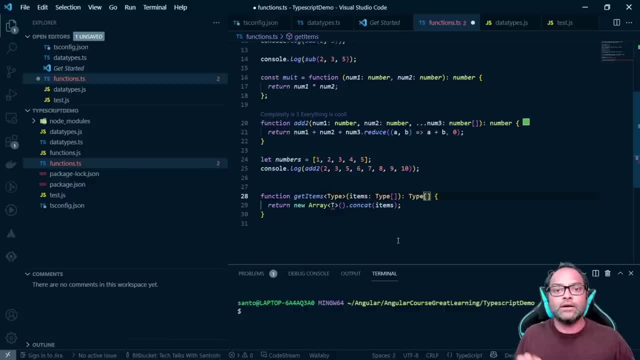 T to type uh, the uh official website of typescript, which has a typescript handbook. they use this pattern so they don't call it T to avoid this confusion. they use type. so we know, okay, what we uh. what we mean is: this is a placeholder, it doesn't mean anything. so, uh, let's try to. 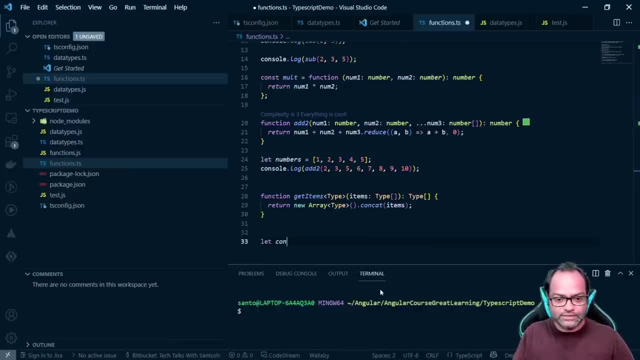 pass some values and use this function. so okay, I'll call it as concat. result is equals to. we'll call get items. and right now let's see what we are doing here. so we are passing the array of numbers and it knows that. okay, we are saying okay, as this number, all the types are. 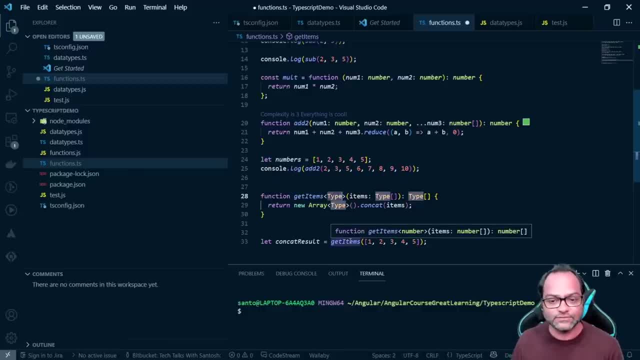 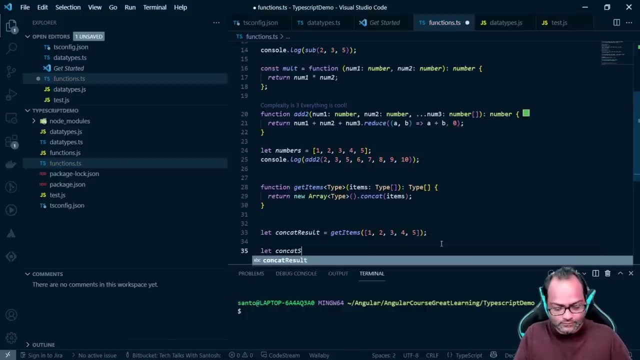 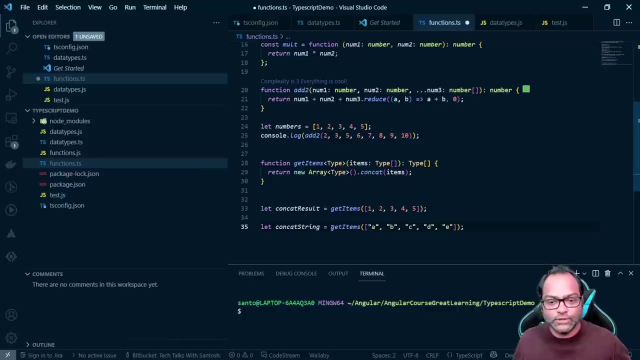 replaced and it is replaced with numbers. so you can see. this is how it generics work, so I can also do. this is equals to get items and now I can pass ABCD and now you can see it will say: okay, the return type is string. you can. 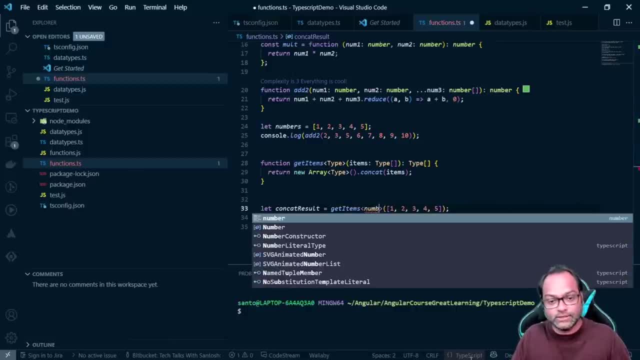 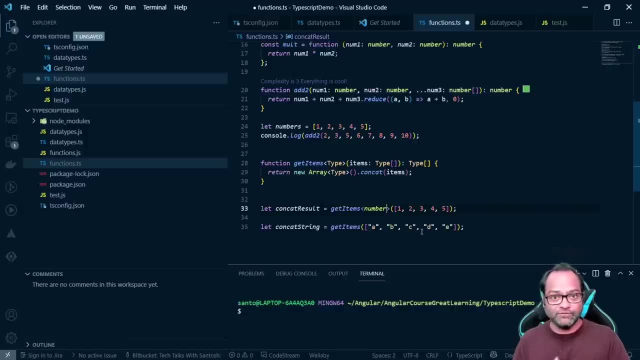 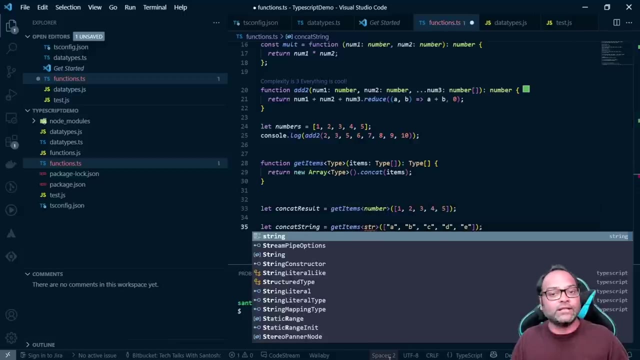 also do this. you can pass the return type- I mean the type T here- so you can say, okay, it will be. I'm expecting to pass number and everything which will be returned should be of type, number, array and same here, so it can infer the values. I remember we spoke about inference, so it can. 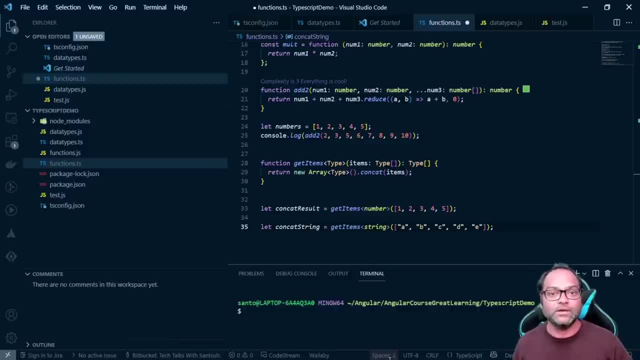 infer the values and it can give you the proper return type. so this is really useful in case you want to create some reusable function which, apart from its type- right, uh, it can, uh, we can- take any type and it can work. so you can do this. you can actually go ahead and create that function as generic function. 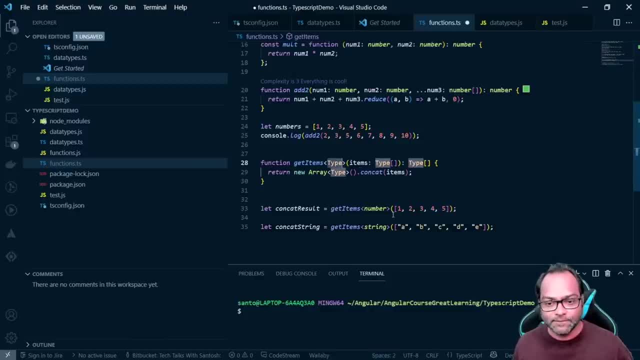 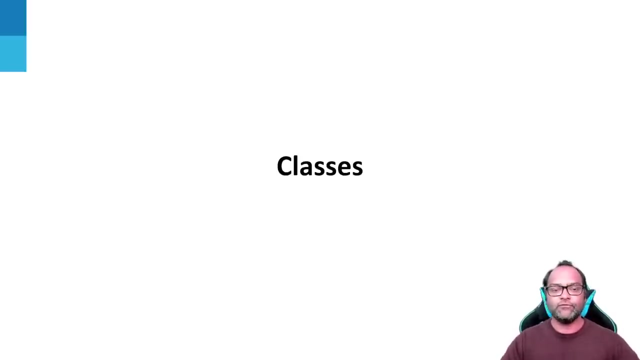 so you can replace this type with whatever you want, whatever you are working with. good, now we are going to talk about classes. if you have very any prior experience in programming, you might have heard about classes, because object-oriented programming starts with classes. you have, like inheritance or polymorphism. everything is around classes in JavaScript there. 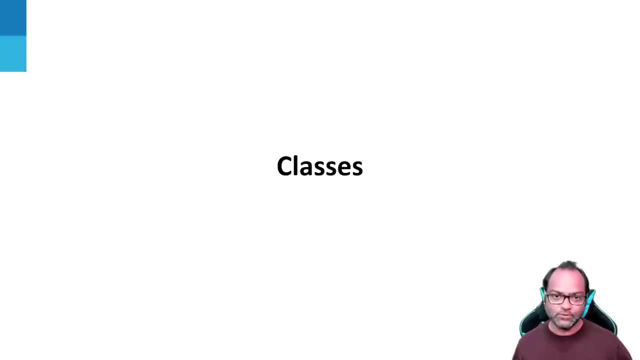 was no concept of classes for a long time. am I wrong? yes, I'm wrong. so there was a way to create classes in JavaScript, but the Syntax was a little bit different and it was- uh, it was, you may know this- something called iffy immediately invoked function expression. so that was equivalent. 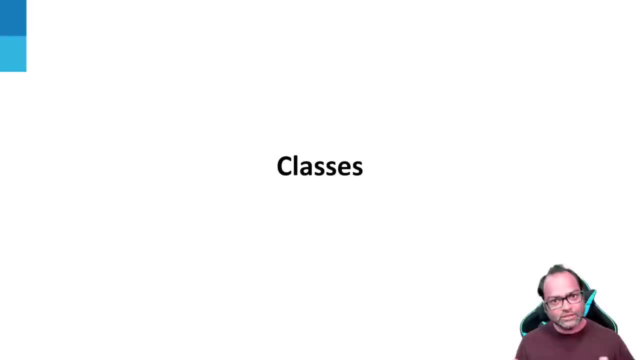 of class in javascript and with es6. thanks to es6, we have class syntax available. so thanks to es6, we have this class syntax available and typescript had it actually before, before even that it was introduced in es6. so earlier typescript actually used to like we used to write class syntax in. 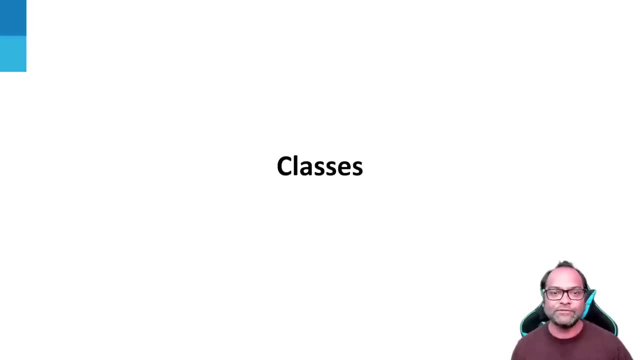 then it used to transpile into es5 and then used to give us iffy function. but when es6 introduced classes, it started actually giving you class syntax. so you will see when we write classes, syntax are pretty much similar in javascript as well as typescript. so let's go ahead and see what. 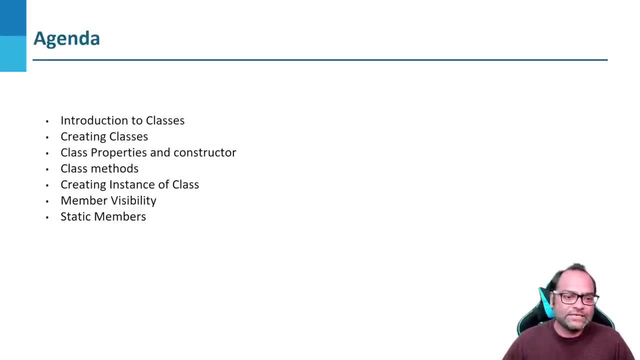 we are going to see. so we will see. of course, we'll talk about classes. we will see how you can create classes. we will talk about properties and constructor. we will talk about the how you can create methods, how you can create instance of a class. you will also talk about member visibility and then static members. so let's go ahead and get started. 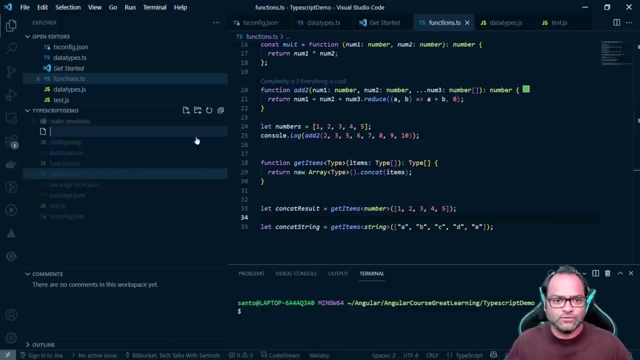 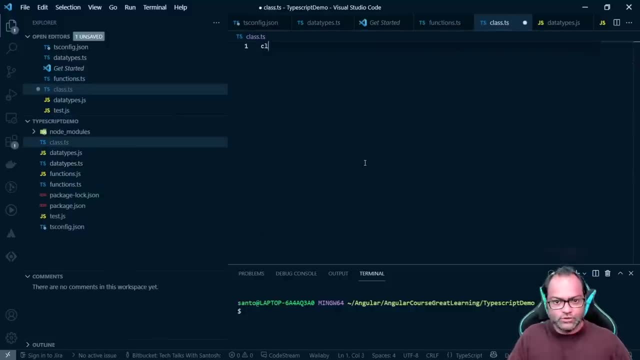 and let's create a new file so we'll call it as classjs. so how you write class, so you will use, of course, class keyword and let's name it as employee. so for naming convention, uh prefer this, uh, pascal case employee. so let's say employee, if i have. 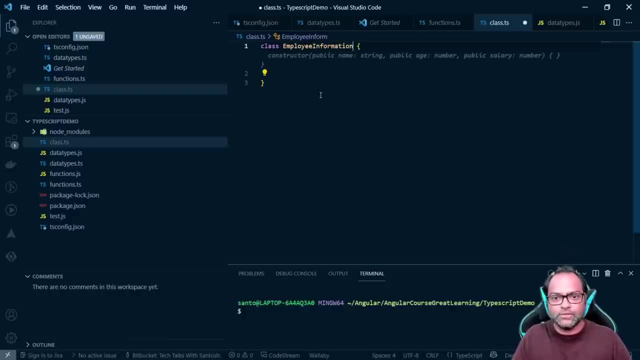 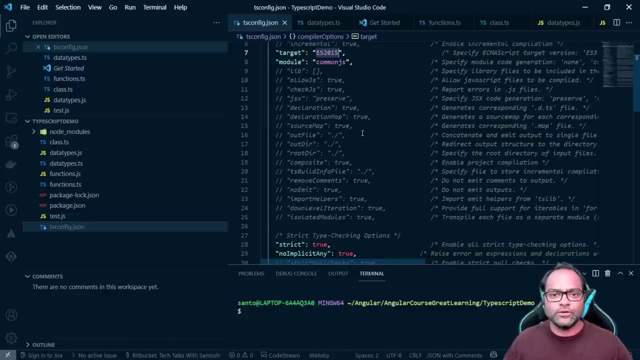 employee information. so i will be capital. so right, this is your pascal case. so right now we have a class called employee. so this is how you create class. and let me go to tsconfigjson right now and remember we changed this target es15. we are saying we are going to support modern browsers, but what in case? 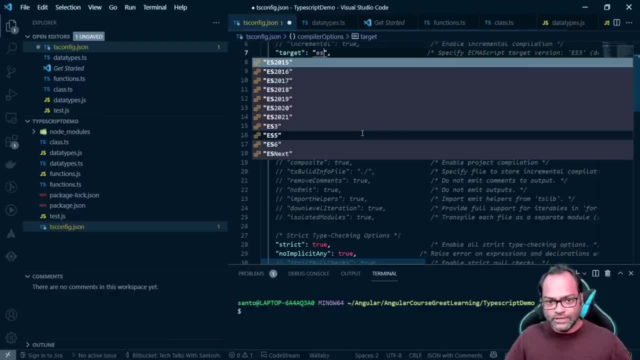 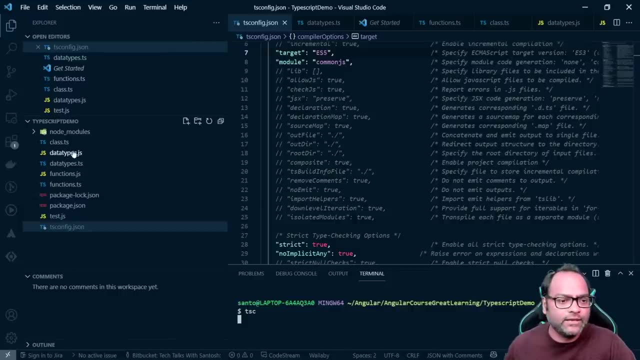 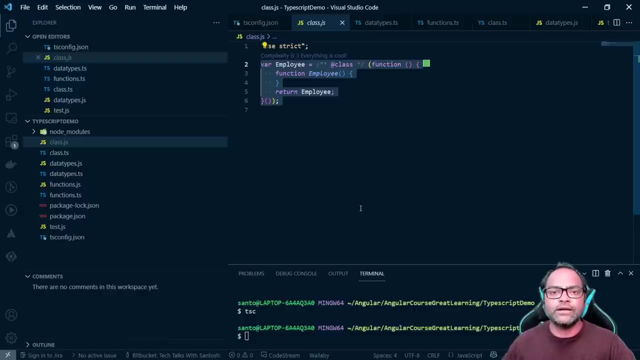 i want to support older browser, so let's see how it used to create classes, or we used to create classes in older days. right in es5 i can say tsc and it will transpile and give us this file so you can see this. this is known as immediately invoked. 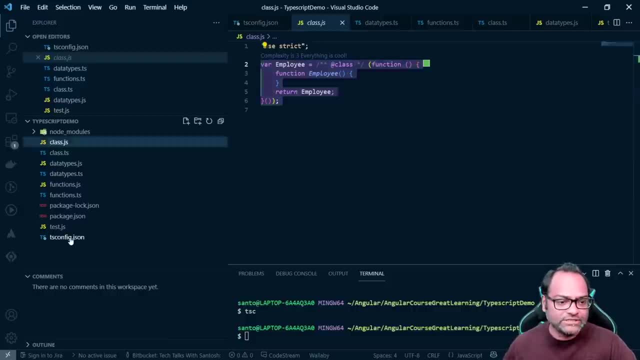 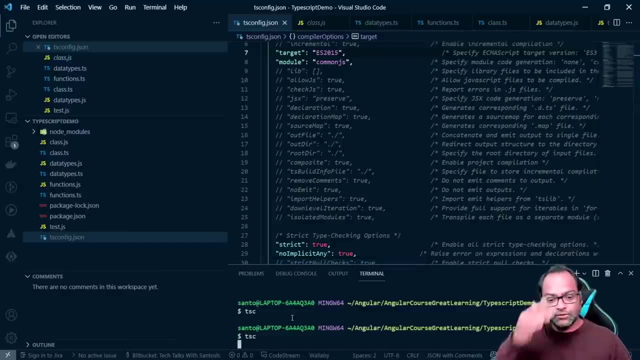 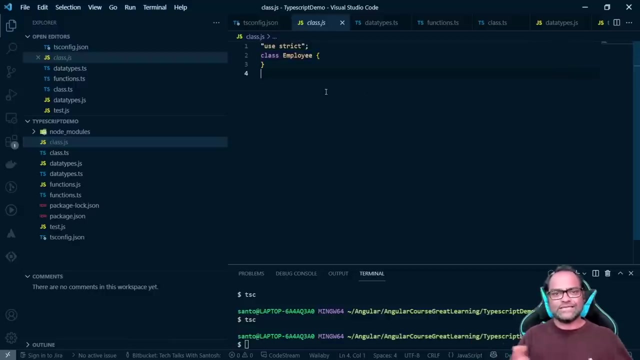 function, expression or iffy. but if i change this configuration to use the es2015 version, which is now supported by all the modern browsers, and you can run dsc again and you can see, okay, same syntax, right. so, class employee, now let's uh, go ahead and see how it works. 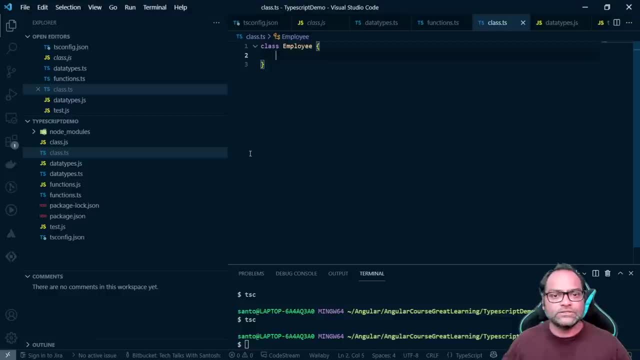 uh, let's add some properties to this particular class. how so, let's say, if we want to have some properties and some constructors, which we generally do, let's see how we can do that. so to define properties, you can create, let's say, id which is type of. you have to give type to each. 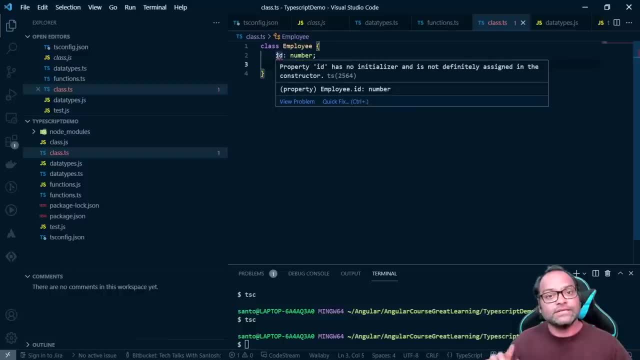 property. you should, and right now, as we are in strict mode, you will get this error. it says id has no initializer and it's not definitely assigned in the constructor. so let's see how it works. in case you have default values, go ahead and do that. otherwise just put this: uh. exclamation. 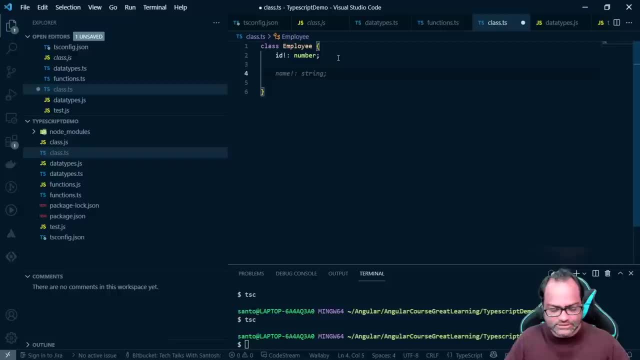 mark, which will uh, which will avoid this error, and we can see a name and we can say address. so this is how you can create properties. but in case i want to use constructor and i want to actually assign all these properties using constructor, typescript has a default constructor. 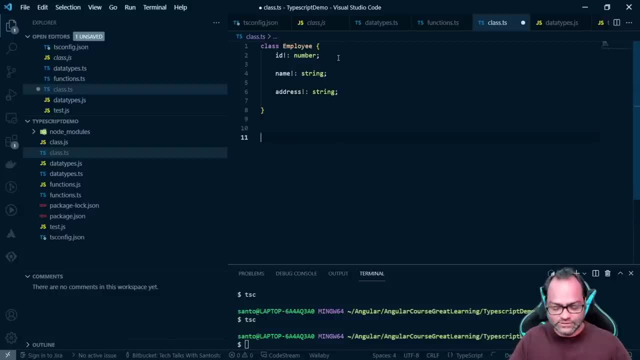 so let's go ahead and see how you can create this constructor. now let's see how you can create this. you can create an instance of this class first, so i'll say: okay, this let emp is equals to new employee. i'll call this employee as john, right, so this employee name is john, and then we can. 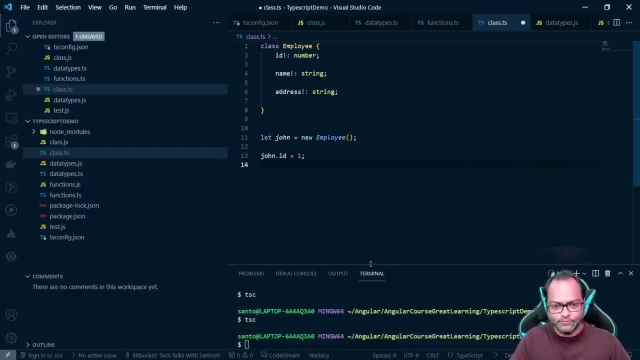 define or we can assign some properties, so i can say: okay, this one name is sean and address is hyper 71. okay, so this, these are the property, these are the values which you have assigned to this particular property, and let's see how it looks like, so you can just: 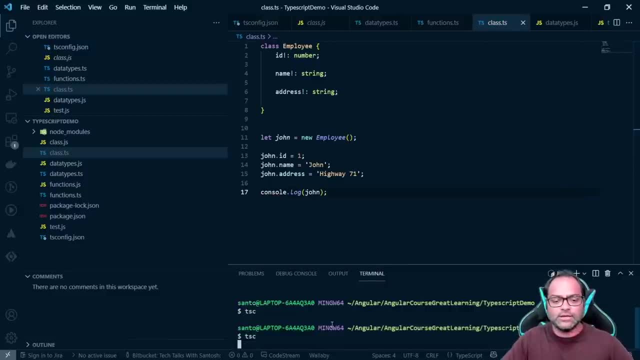 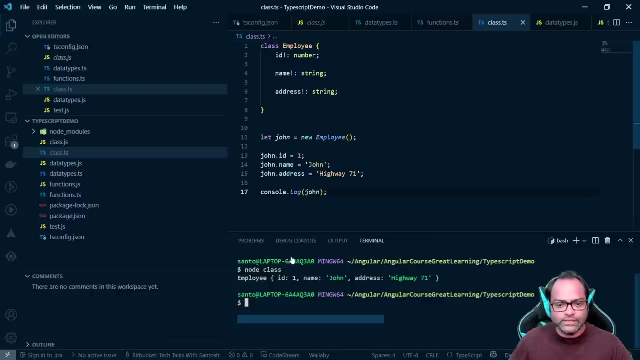 say consolelog, john, and let's transpile this file tse, and let's run it using node and you can see it gives you a employee object, right and it's. it is giving you all the values: id, name, address. so this is how you can create a class and assign its values here. 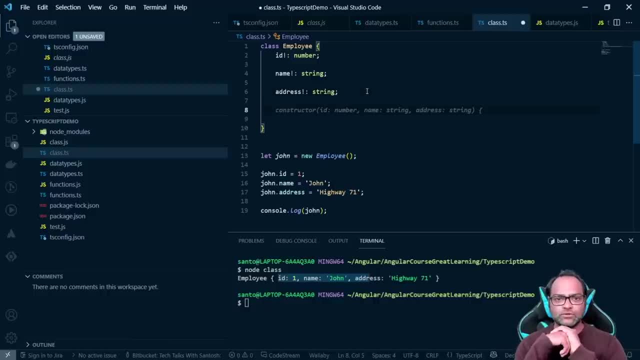 okay, now let's talk about constructors. so constructors are something which will be which will be responsible for creating an instance of this class. so how you can use constructor? of course, by default, there is a default constructor which is available. you don't have to in case you don't want to, or you can have parameterized constructor. so 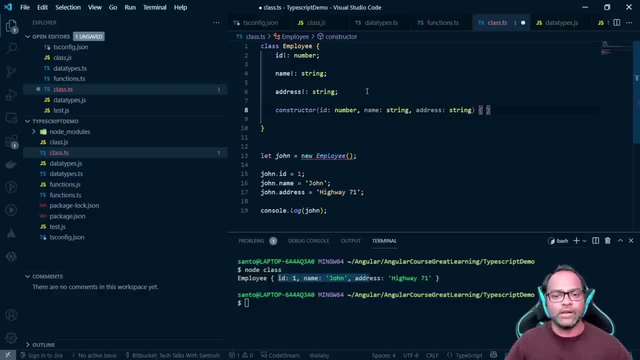 in other programming languages you can actually have parameterized constructor as well as default constructor. in typescript you cannot have both. you can have either default constructor or parameterized constructor. so here let's try to actually do that. i'll create another constructor, function constructor, so you will get an error. so here you can see it says multiple. 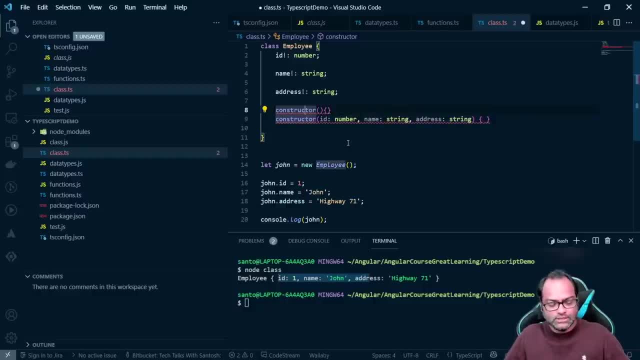 constructor implementations are not allowed, so you cannot do this by using constructor. of course we- uh, we can avoid this, like in case we have default values. right, we can do something like this. i can say: okay, this dot address is equals to address. you can see, as soon as i do this, the error will be gone. 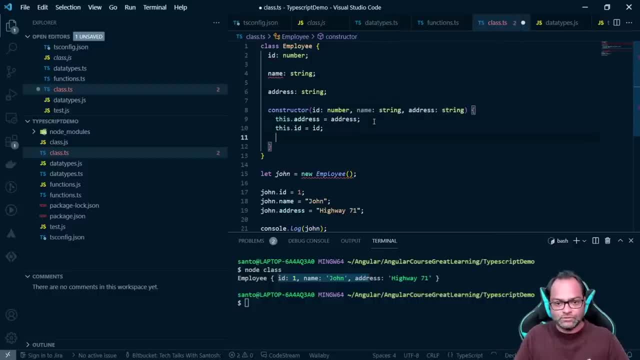 and then i can set this dot id equals to id and this dot name equals to name. but once we do this, i mean what we are expecting is we are supposed to pass this properties while creating the instance. so when we are getting the instance, you can see at line number 15, and we started getting the error as well because we are not passing those. 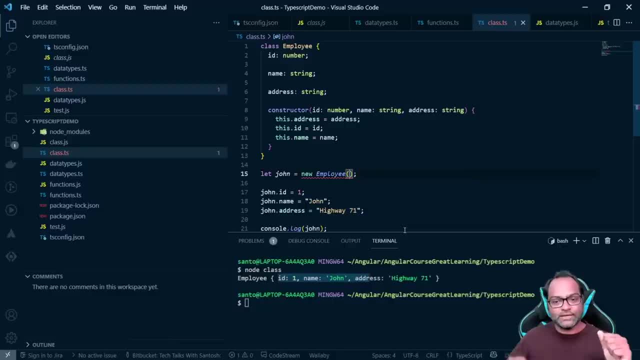 values and it is expected that whenever you are creating an instance, you have to pass the value. so rather than actually passing this values here on line number 17, 18 and 19, we can go here so we can say: okay, one comma, john and uh. address is hyphen 71 and we can remove this. otherwise it. 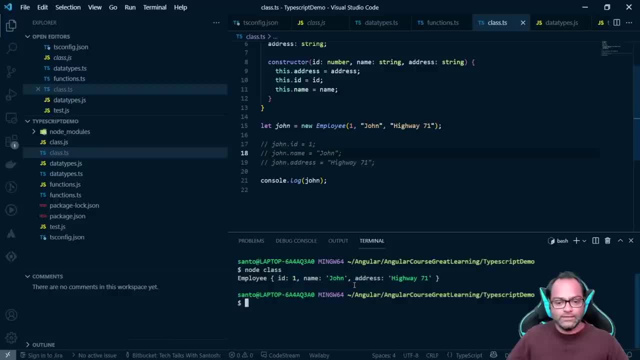 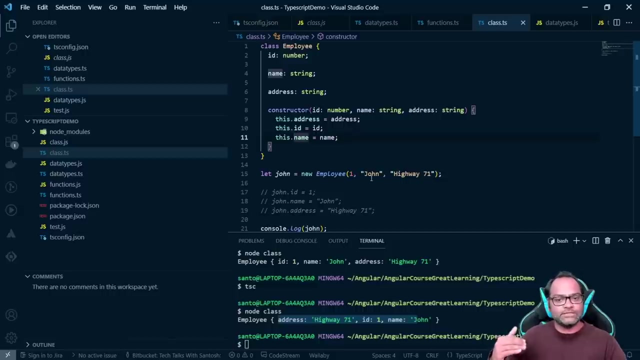 will just overwrite the values which we don't want to and let's run it again. so i can say tsc, and now i can just note and you can see you have the properties right. so same values which was assigned here is available. so this is how you can actually add properties and this is. 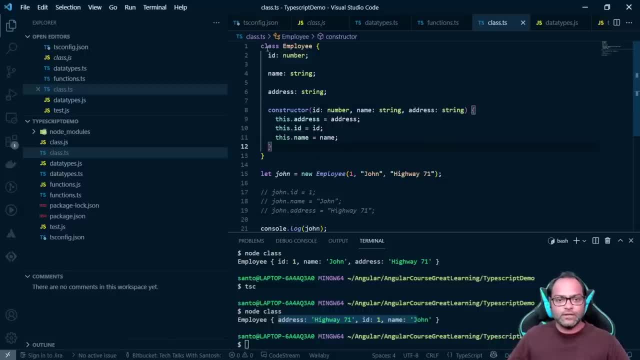 how you can create a constructor function. now let's talk about methods, how you can add methods to your class. to create methods, you can just give a function name. you don't have to use function keyword. so i can say, okay, get name with at this, and what i can do is i i want to actually have a written type, as i said we should. 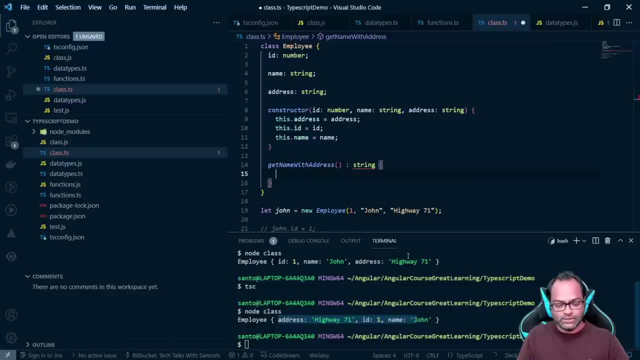 have a written type here string, and i will say, okay, this is written, uh, this dot name plus this, this dot address. here actually i want to introduce one more uh syntax to you, so here we can see: okay, we are passing this dot name and then we are passing, we are concatenating two strings, basically. 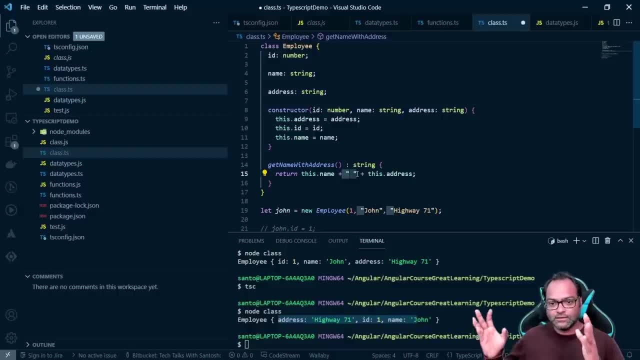 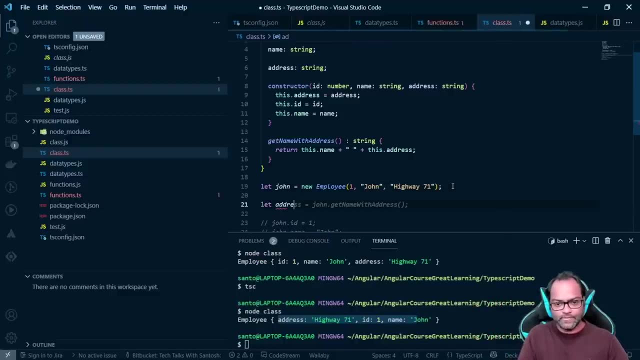 so we have this dot name and then this uh name will be john and uh, then his address, which is highest highway 71, let's try that out right. so i'll say: let uh address is equals to john dot, get name with address, and then we'll. 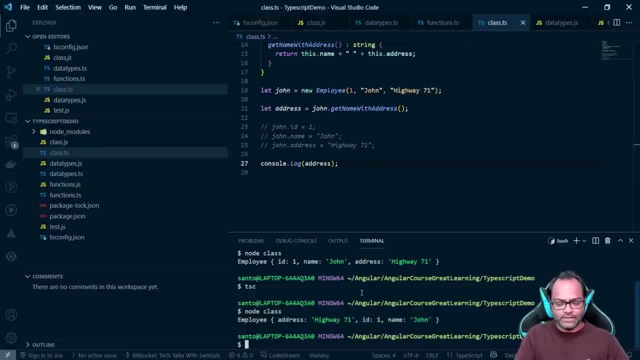 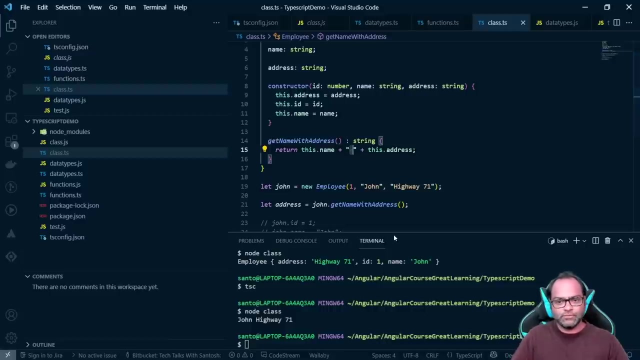 just do consolelog here on line, but 27 and let's do tsc and we have this john highway 70. but this way of concatenation is really uh buggy sometimes because your, you may miss this. so it happens, it happens, it happens with everyone. uh, it happens with me it. 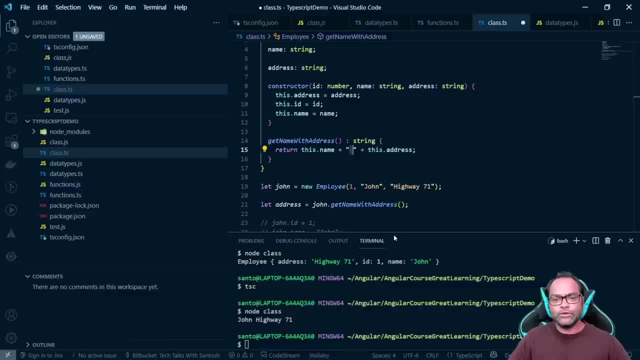 happened with me uh, in past as well. so what you can do is you can actually uh use the another, you use another syntax which is, uh, string, literal. uh, you can actually do something like this, so you can say uh in single quotes, so you can uh use this, um, this key, which is field, which is known as. 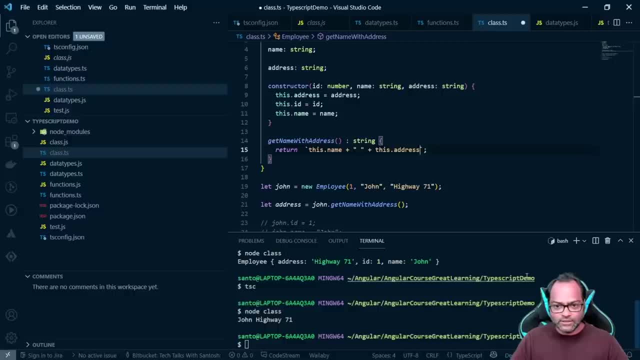 tilt. you can press this: uh, without shift right, so looks like single quotes, but it is not, and then you can put it inside the dollar and curly brackets, so variables you can replace with curly brackets, and here also i can do same, so i can say dollar, curly brackets. 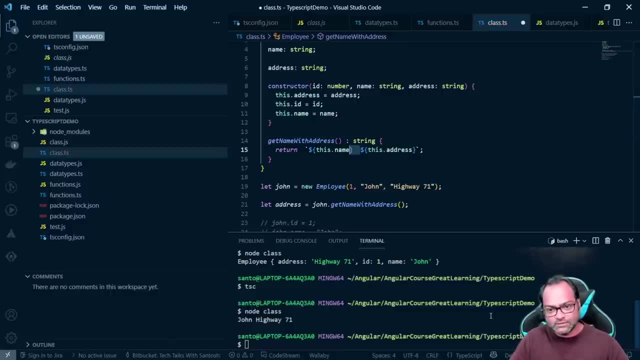 and now you can see i have a space here. i don't have to manually put a concatenation sign- which we did earlier and do that, so i can say, uh, john stays at hyper 71 and let's see the output. and this is something which you can do in angular as well, so it's not like something. 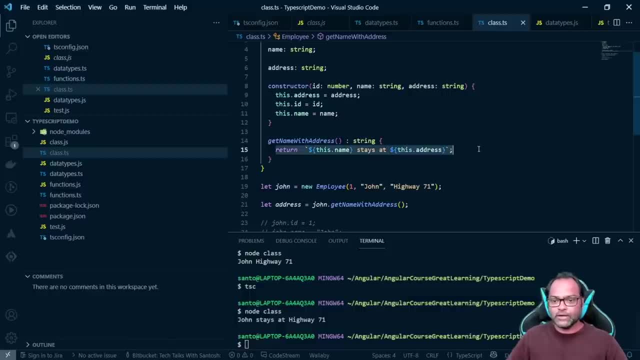 specific to typescript. i mean: uh, you can do where, uh, you can actually go ahead and utilize this code in your real-time application. so, using this string, literals, so you can see john stays at 7-1, no need to actually go ahead and concatenate using plus sign or unknown, and you don't miss your. 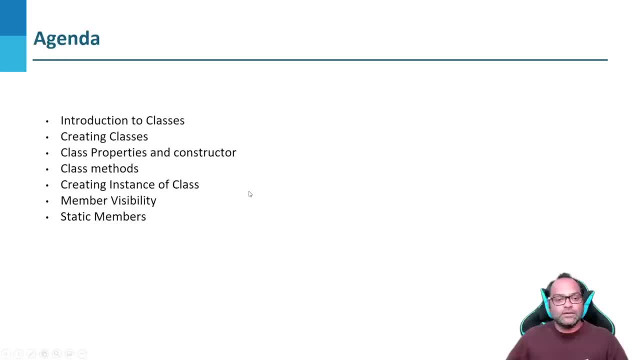 spaces, right, that's. that's a cool thing about it. now let's talk about creating instance of the. so what we learned so far is: we created a class, we created properties and constructors. now we added properties, we are also added constructor. we've added a method. we created an instance of class. this is how you do it right, so you'll see. 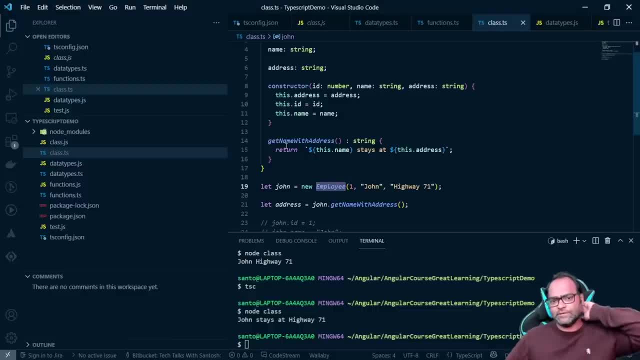 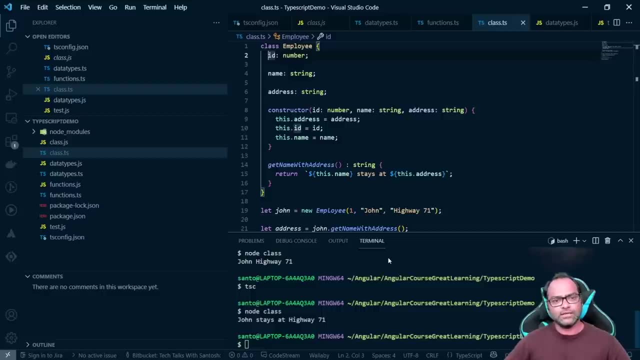 using new and class name. Let's talk about visibility, right Member visibility. here You can see you have properties, ID name, address. But before that, I think I'm used to actually talk about why to create classes. That's really important, right. 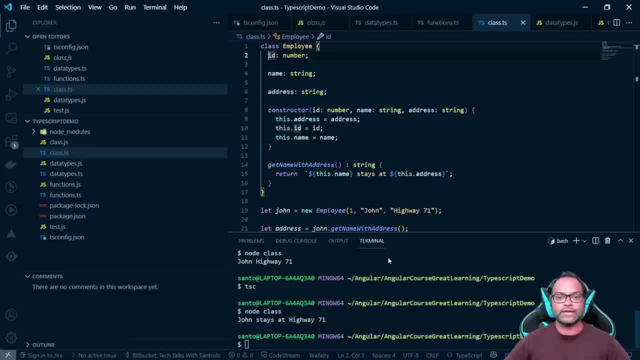 So, in your application, what you are going to do is you are going to create a lot of code which will contain your business logic: How to actually write those business logic, or where to write those business logic. That's where classes comes really handy. 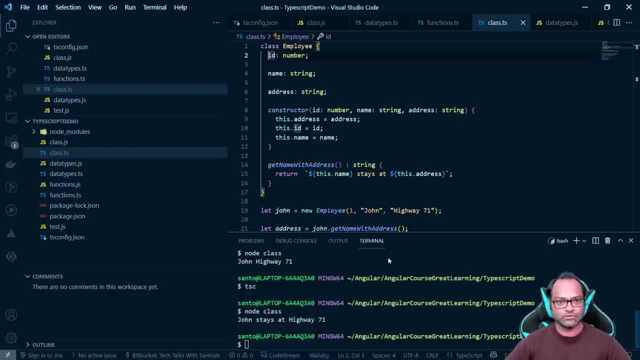 So a class will be responsible for, like, handling some business logic which you will be writing, For example, let's say, in Angular. we are going to use classes for writing services which can have, like, getting data from your backend and displaying it on your front end. 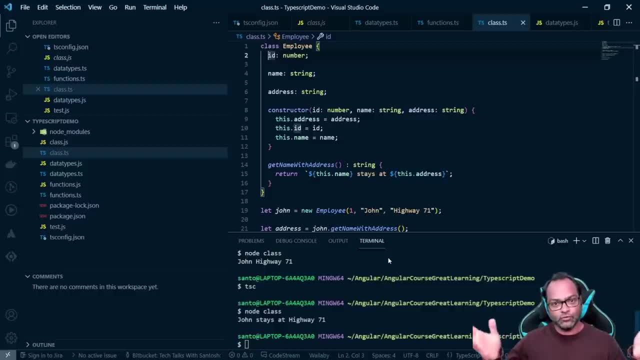 We'll be using it for components which will be kind of your view. So it needs some backend, right? I mean, it needs some class to actually give the data back to your HTML. That's where we'll be using classes, So it will just wrap your entire business logic. 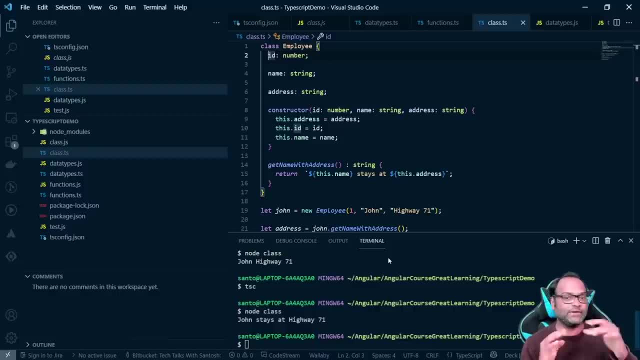 You are going to write your business logic into classes and you will have like tons of classes right, Different classes where you can have different logic. For example, if I'm writing some logic related to getting the data from my backend for all the rooms I own, 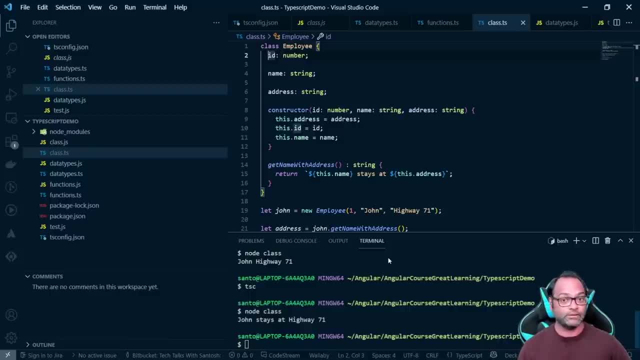 For example, if I take an example which we are going to go and implement in this course, we are going to create a hotel management application, So where, let's say, you have like a lot of rooms available so you can write a class to get those room data. 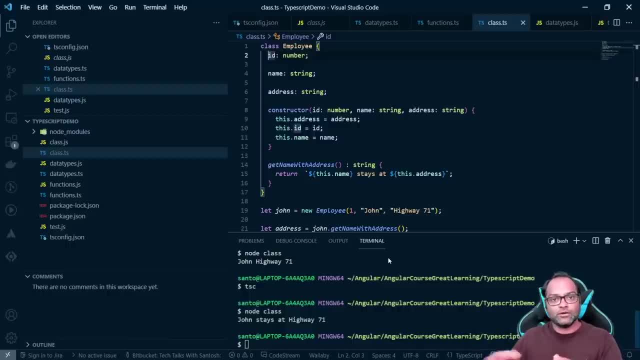 and display it on your front end and assign, or you can have like logic to assign your rooms. Those are the different logics which we will have, So those logics will actually go into your classes. So classes makes like splitting your logic into smaller chunks, right? 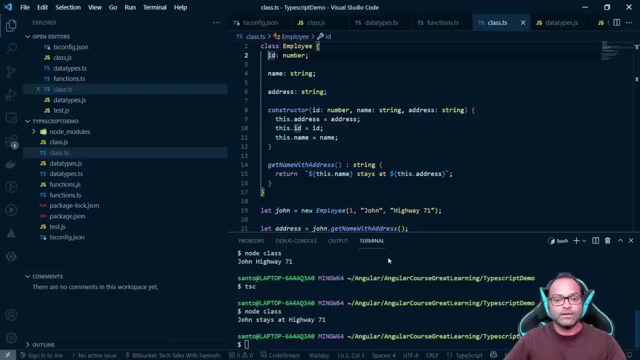 That is what your classes are going to make it possible, And you can do a lot of things. You can do a lot of stuff with classes, which we'll see Here. let's say, we have right now ID You can actually create. this is private keyword. 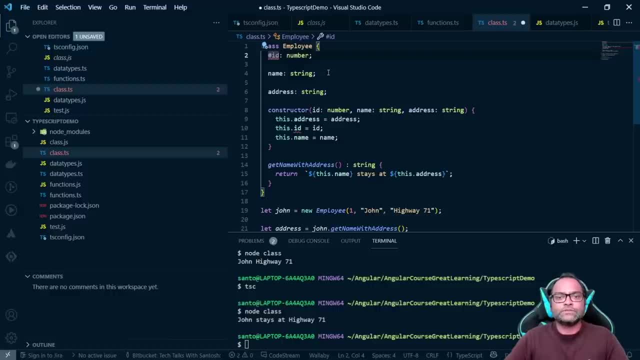 which is introduced in new version of JavaScript and now supported by TypeScript as well. Or you can also use private keyword, but I think you should not anymore, because it's the native when you support it. So you can say hash ID. Let's see what it says. 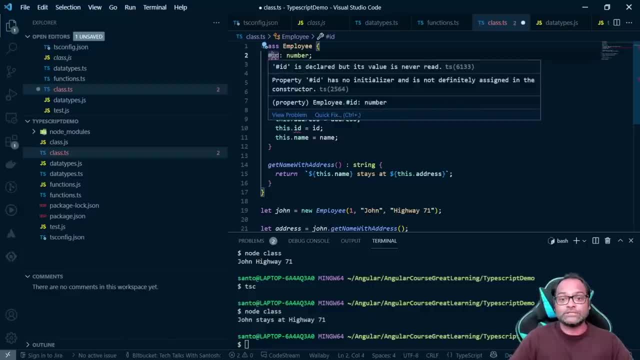 So it says hash ID is declared but its value is not. It is never read because it says, okay, it's a private value. sorry, private variable. You can see now we have actually started getting this error here as well. So I can say private or I can just use hash ID. 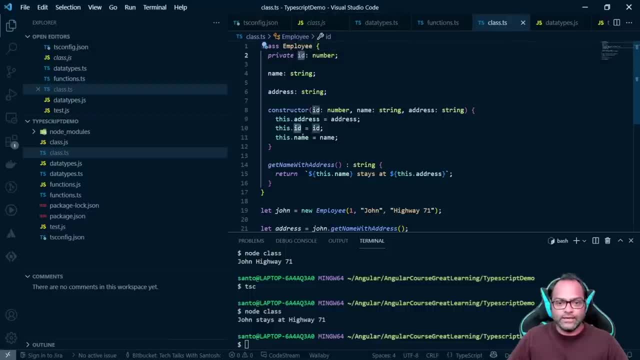 in case you want to keep it private. So here you can see private ID and then with private- sorry, private- variables, you can actually assign them into your constructor. So if I keep this one hash ID, so what I have to do is I have to go ahead. 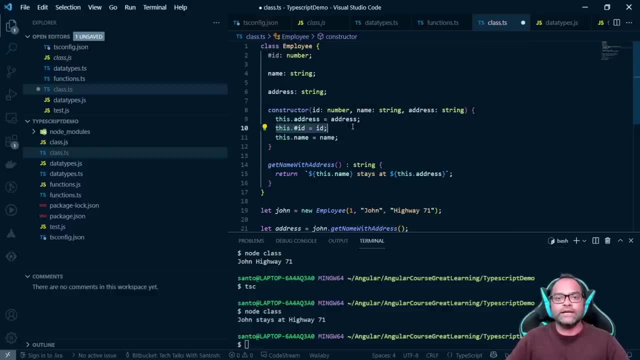 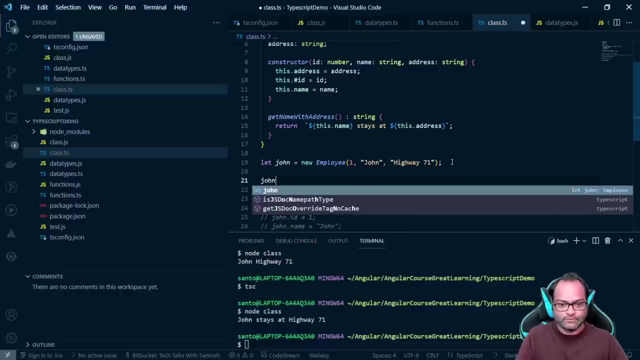 and change it here as So I can assign this inside my constructor. If I try to access the properties, you can see I'm not able to access ID because it's a private. it's private to the class and we won't be able to access. 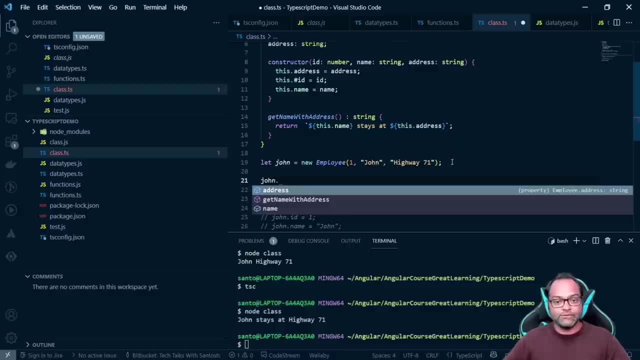 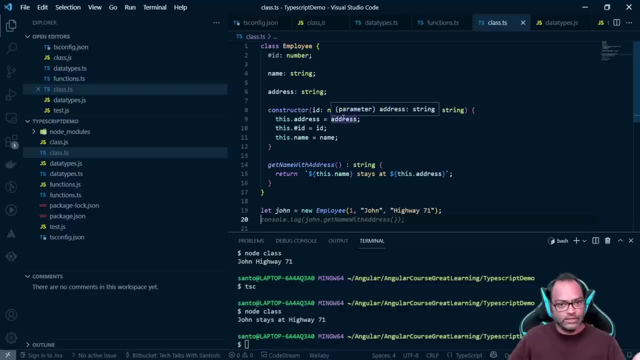 whenever we create a new instance of that particular class. So that's the private property for you And prefer now if, as you will be using probably Angular 13 in future, I mean by the time this course gets released- you prefer hash ID, which is like the native syntax. 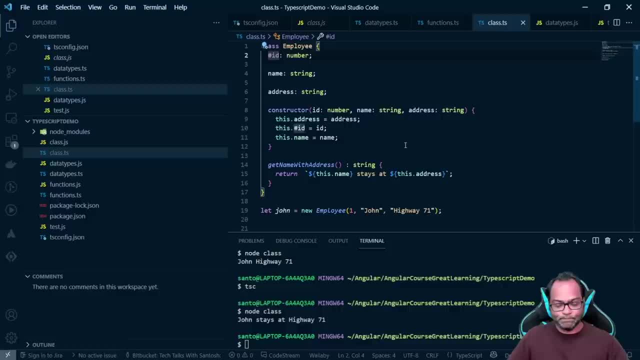 for creating private variables in JavaScript. So this is private By default. all the properties and all the classes are public. You don't have to mention that. You can also make it protected. So you can see: okay, now I have made it protected. 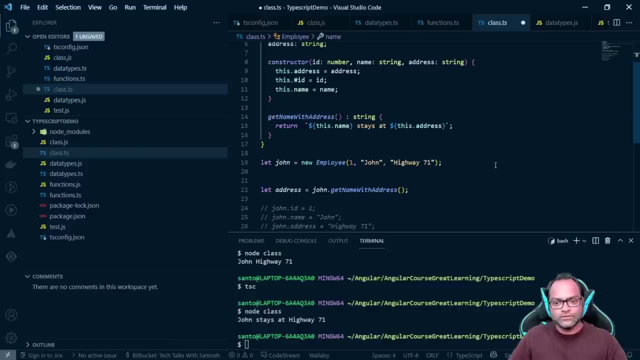 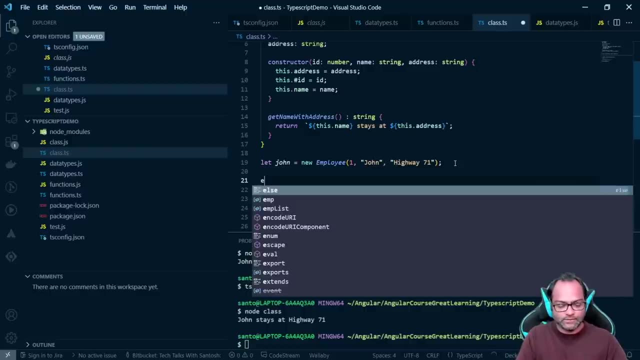 So why what protected does it is useful? So why what protected does it is useful? So why what protected does it is useful. In case you want to extend this particular class, So let's create another class- I'll call it as class manager- which extends employee. 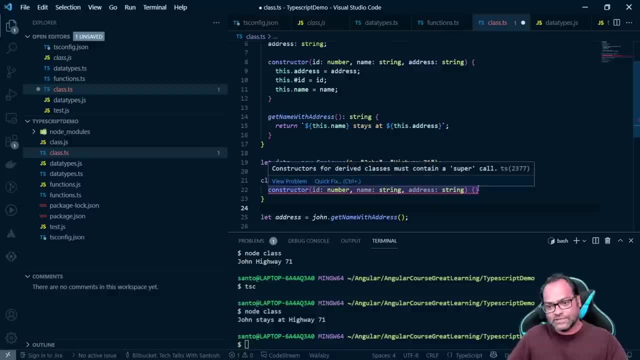 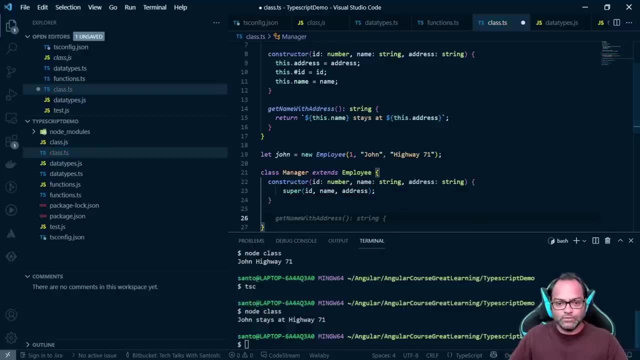 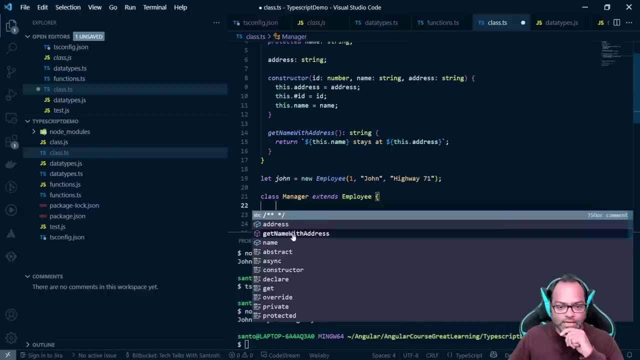 So here it says constructor for derived class. Okay, this is something which is required in case we are extending. So we have to call super and this is it Now. here we can actually access all the properties. So you can see, I can get address and name properties. 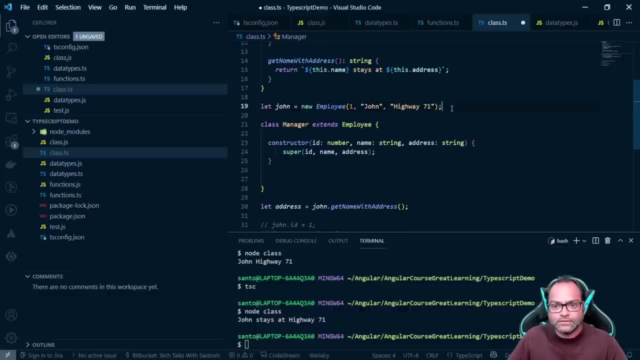 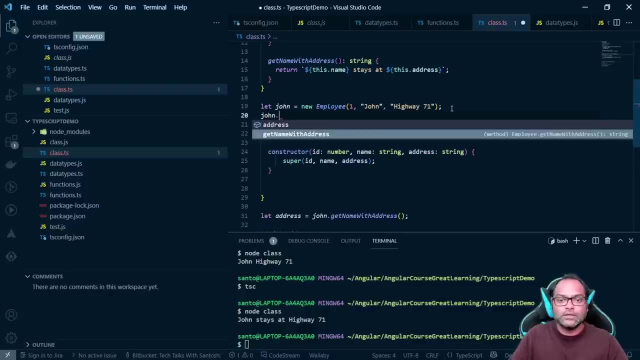 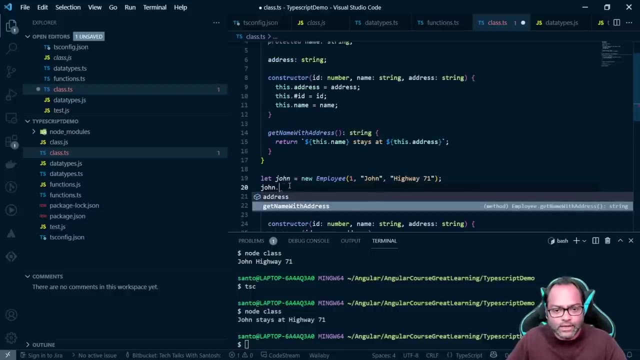 which will be accessible here And but you can see, whenever you create a new object you won't be able to get. I mean so protected is something which will be available within class and the classes which extends this class. 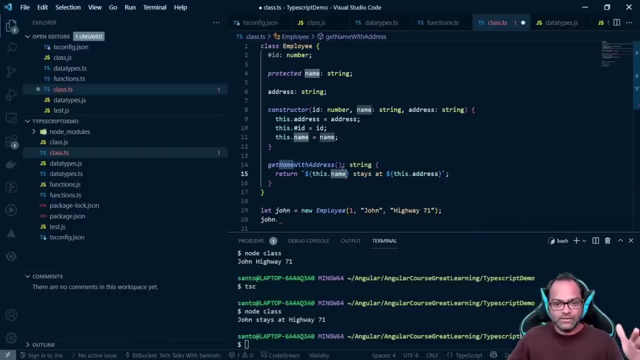 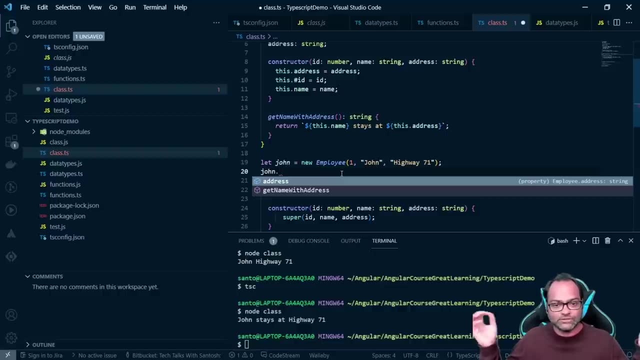 So right now I can go ahead and access this name inside my class as well as the class which extends it, But once you create the instance, you can see it's not available. It's something which is not visible to my instance. 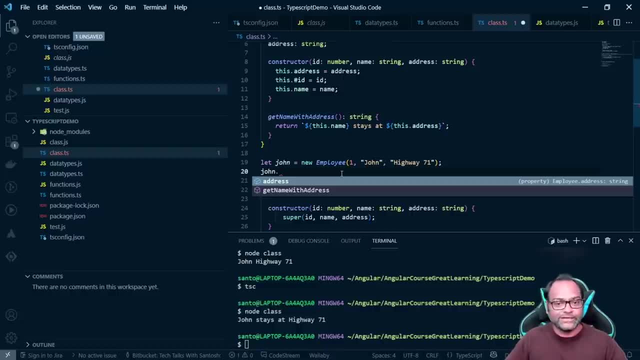 a public instance which is created. So this is how you can actually use protected classes between like, in case you are trying to extend. This is also known as inheritance in other programs. This is also known as inheritance in other programs. This is also known as inheritance in other programs. 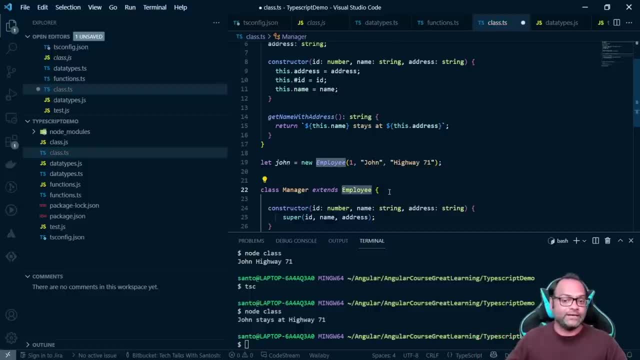 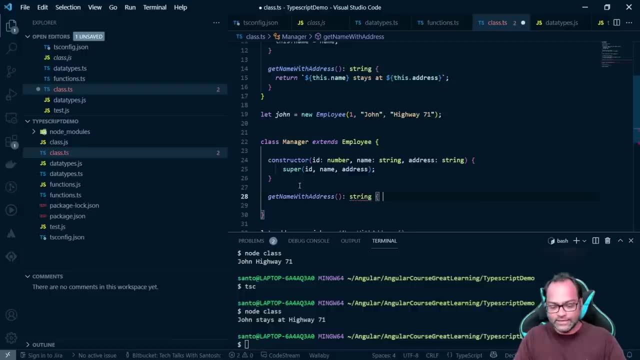 Or OOPS concept, So you can. you also call it as inheritance, So you can also get access to all the members. I'm sorry, methods as well, So I can actually create this get name with address, but here I can say this: manager. 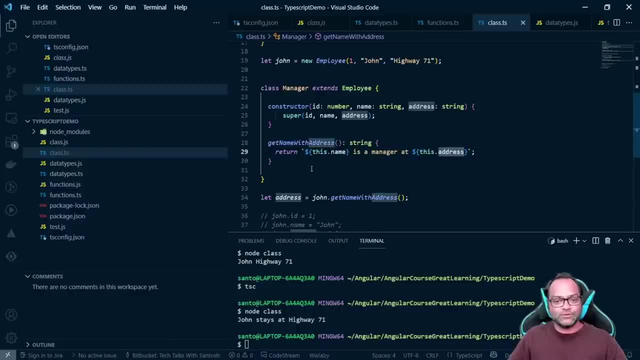 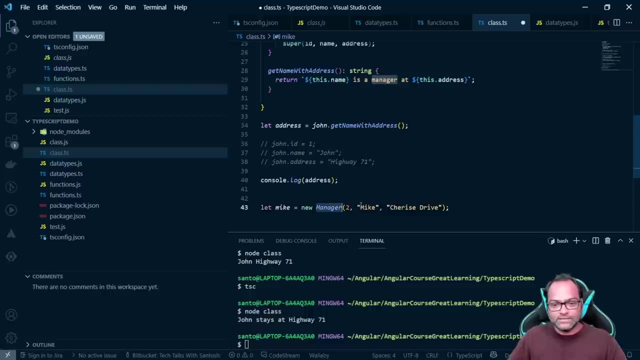 this: whatever name is the manager at this particular branch, right? So this is really nice. So I can say: okay this, let's create, let's create a new Mike. So Mike is a manager who stays at CherryStripe. 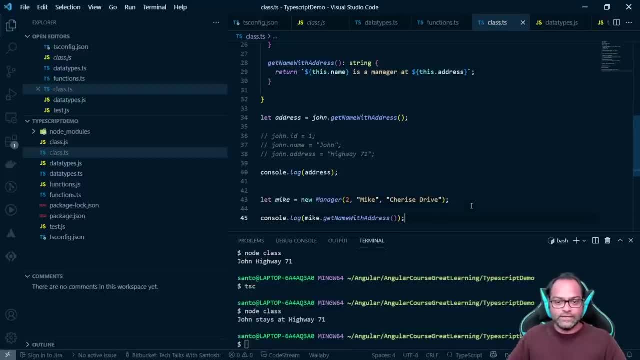 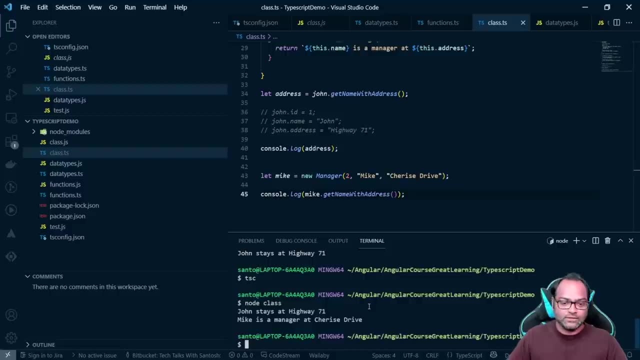 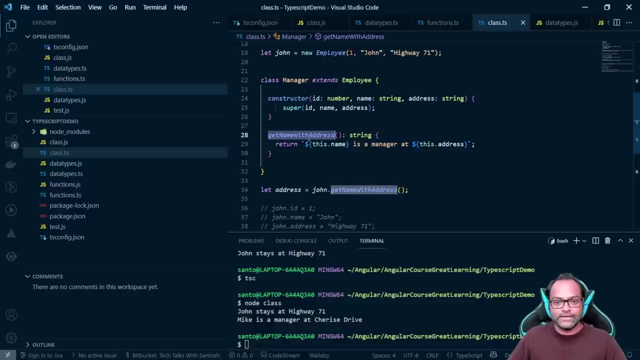 and I can do consolelog and get name with address. Now let's see, We created an instance and then we have actually a new. I mean, we have implemented this. my manager class actually implements its own method, which is called get name with address. 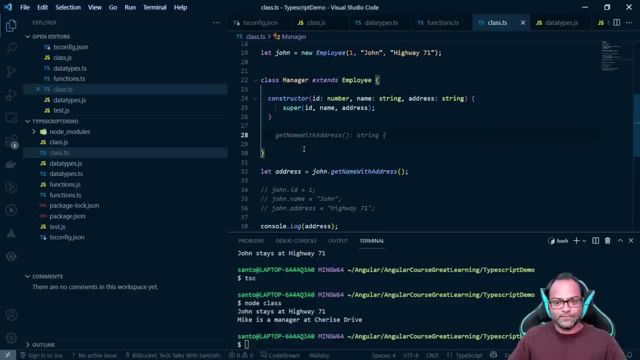 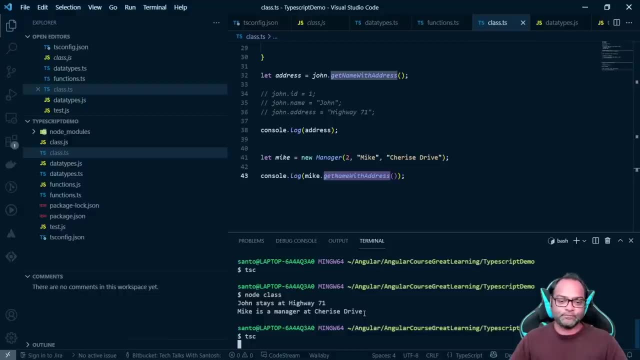 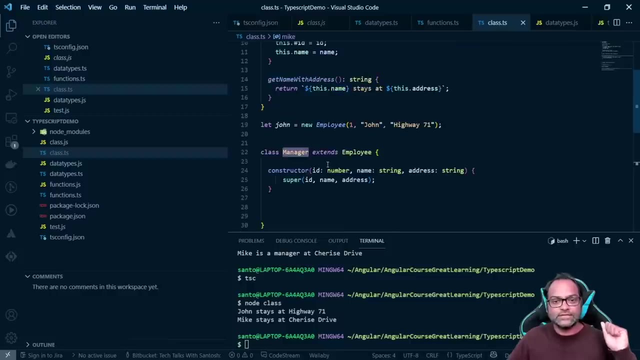 But what in case I don't do this, Let's do that. You can see, I can still call. get name with address. What happens now? So in this case, what will happen is: your manager class knows that. okay, this method exists in my parent class. 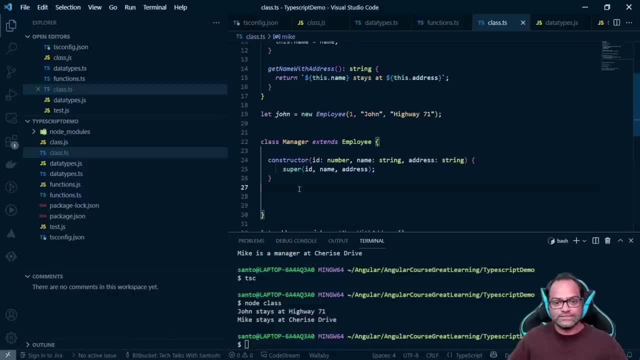 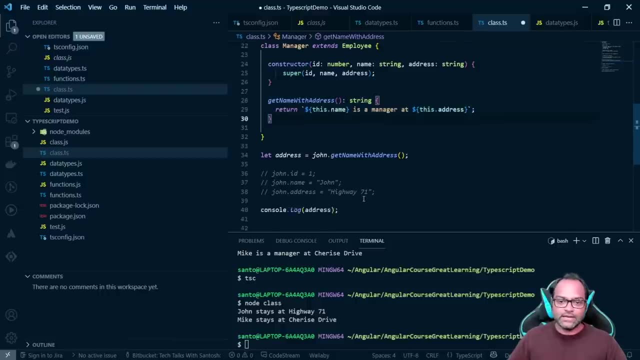 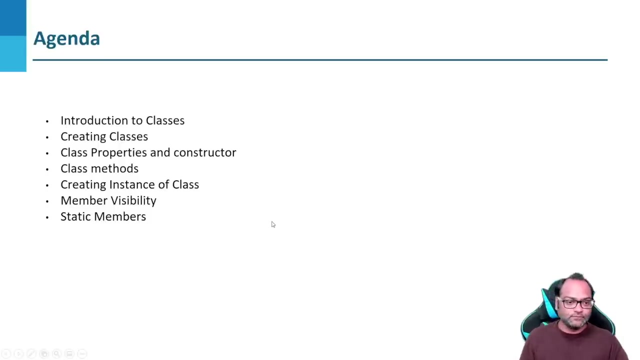 So it will call the parent class. So this is something which is really nice about inheritance: You can achieve this and let's roll it back. So we have its own function as well and we have one implemented by manager. So this is from member visibility. 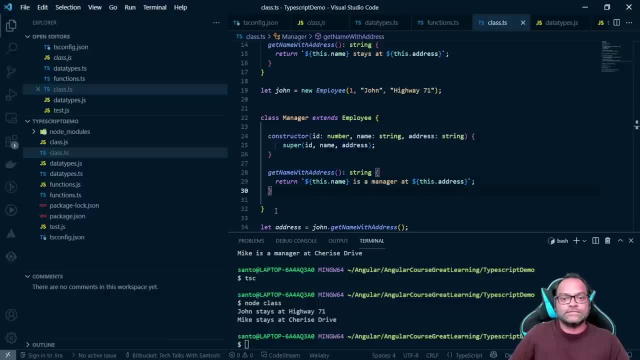 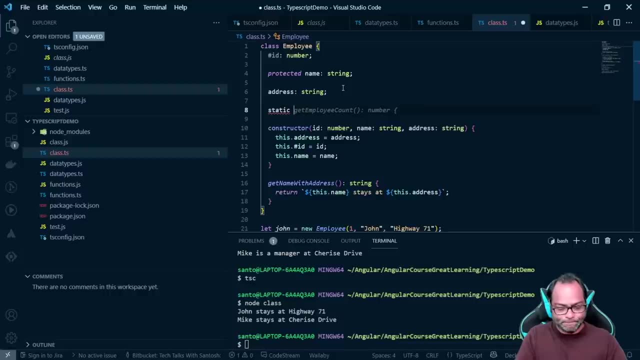 and you can have static members as well. Now it is allowed. So let's see Static members, let's talk about it. I can say static and should I create a method? Let's create a method And I'll say: return 50, right. 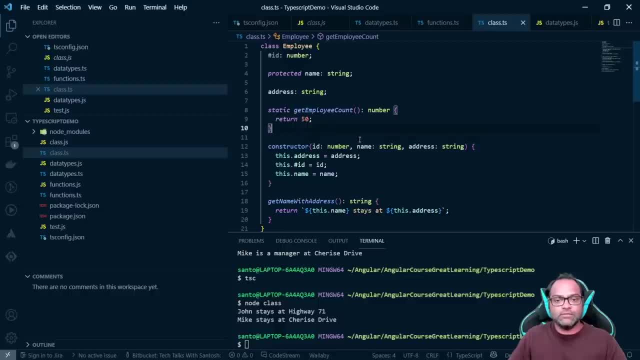 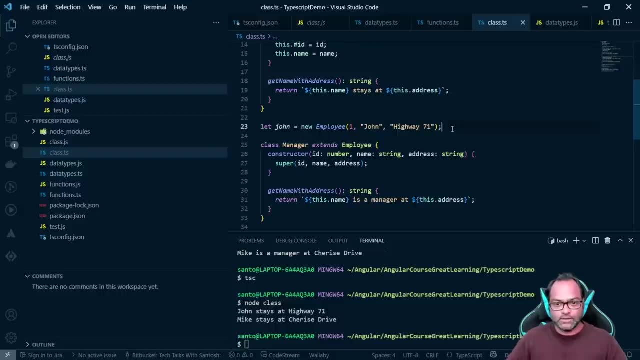 I'm just returning a number. So with static members, static members are something which can be accessed with the class name. So here let's see what I'm referring to So I can say: john, You can see it has address and get name. 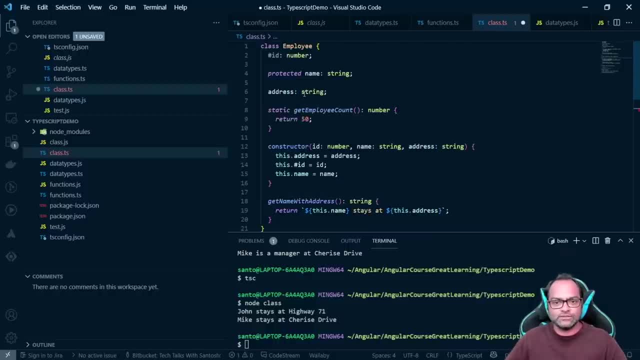 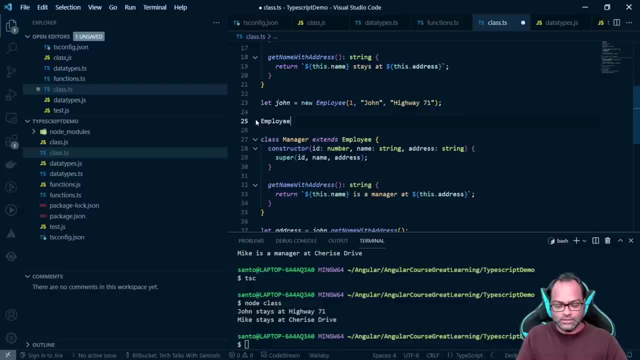 get name with address. Where is this particular function, which is get employee count, So you can do as employeegetemployeeCount, So you will be able to call this particular method on the name itself without creating a new instance? So this is what happens in static. 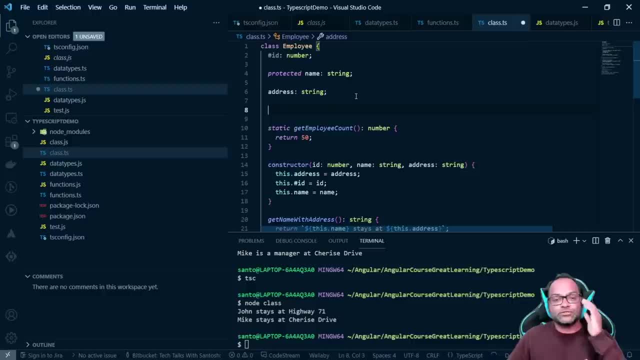 I wanted to show you one more thing. Yeah, I wanted to show you getters and setters. So this is something which is widely used in, you know, in the cloud. So if you want to use programming languages like Java and NET, you can use getters and setters. 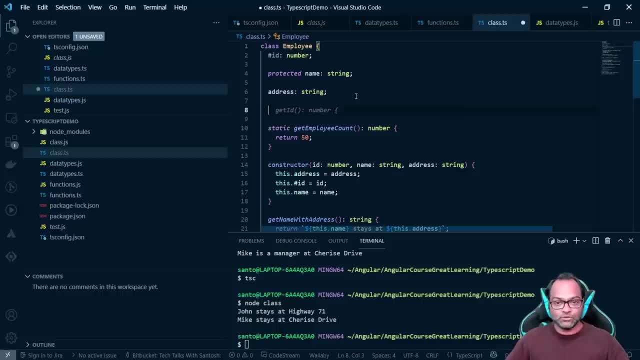 You can also use getters and setters in TypeScript. So here I can say: get EMP ID. So as of now, if you remember, EMP ID is a private variable, So it cannot be used outside. You can. it cannot be accessed outside. 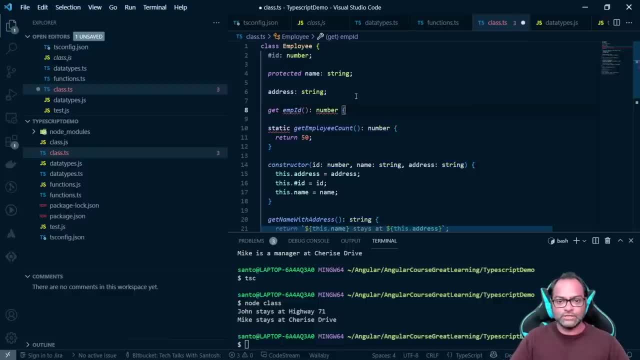 but what in case? I want to access it. So I can do is I can say, okay, this is a getter method and I can say: return this dot hash ID. Similarly, I can say getter method. Similarly, I can have a setter with same name and peer. 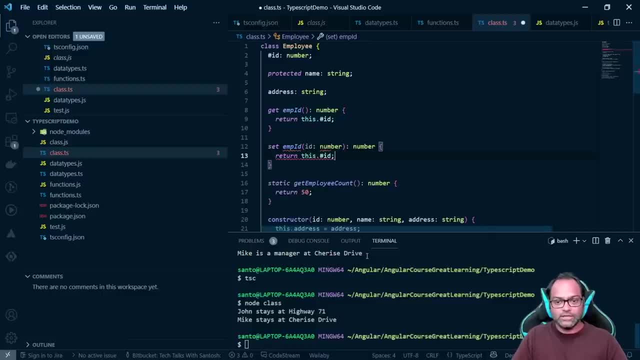 I can say: this will be ID, which is type of number, And I can say: this dot ID is equals to ID. I'm just assigning it, So I don't want to return anything. I can say: okay, this, mm-hmm right. 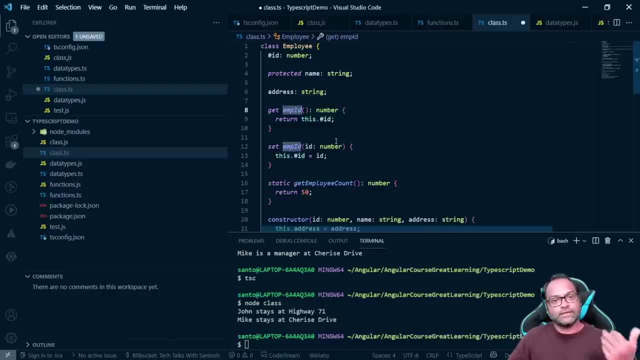 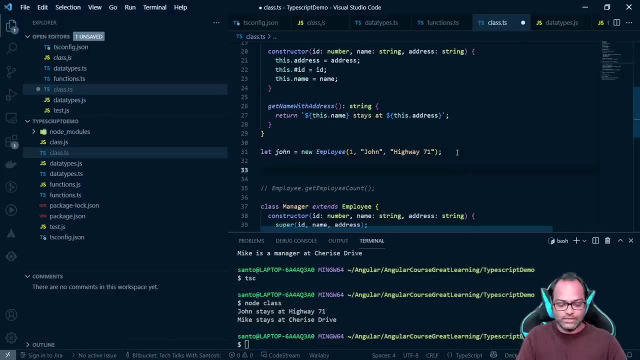 So this is a setter which will assign the value, And this is a getter which will get the values. So now, let's say, let's do this, And I just said, John dot. EMP ID is equals to a hundred, So I'm just then changing this employee ID. 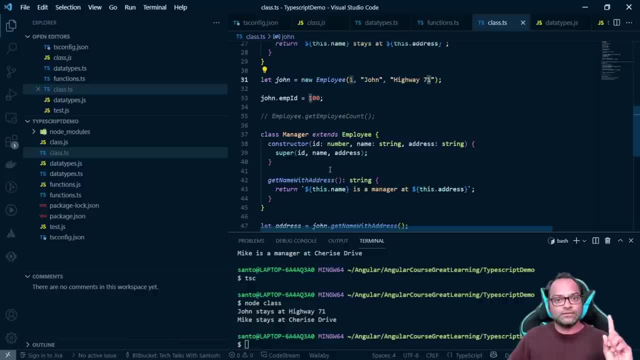 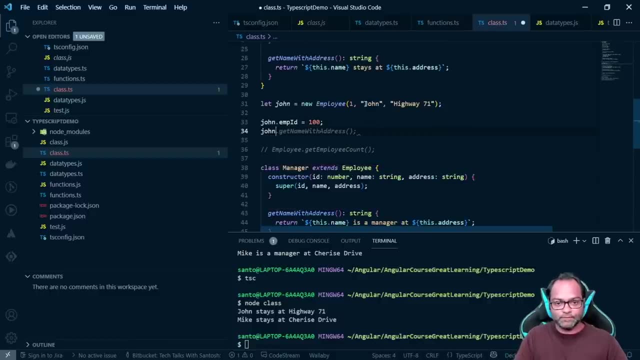 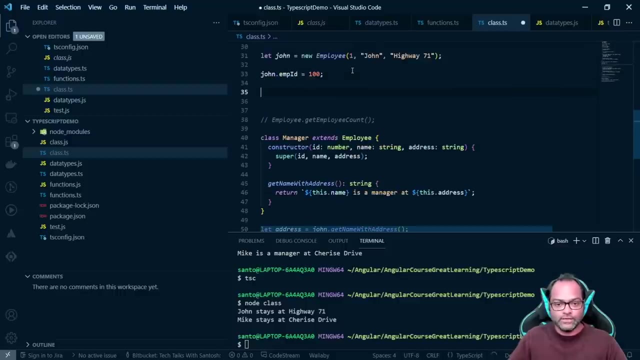 which was assigned as one to a hundred by using setters. And here you have John dot. it says it will be available on the instance itself. So I think we already have console dot log. No, we don't have. let's add console dot log. 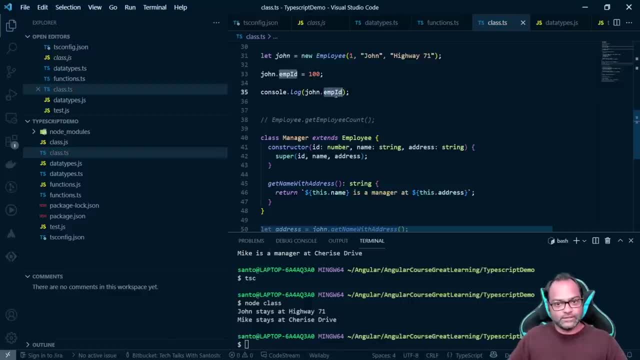 John dot EMP ID. So I think we already have console dot log. No, we don't have. let's add console dot log, John dot EMP ID. So what we are supposed to get it here. So as we are calling it, it will call the getter. 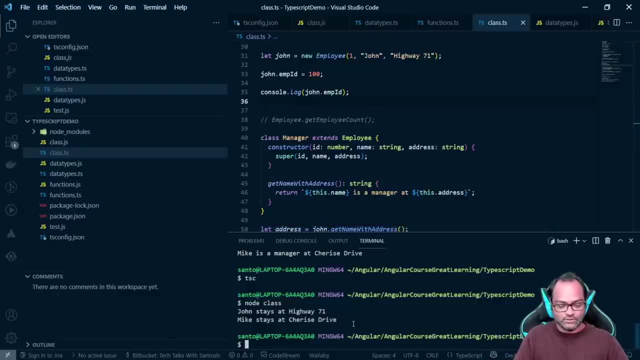 So we'll get the employee ID, which is a hundred. So let's clear and call this again And then call node, which is: note she, I'll be a getting hundred. So getters and setters. it is also possible, in case you have like, hang off using getters and setters, that they are. 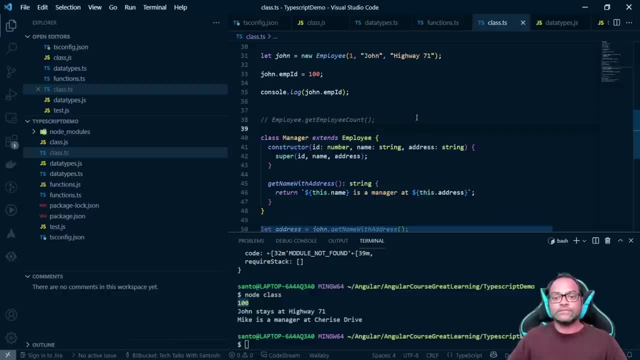 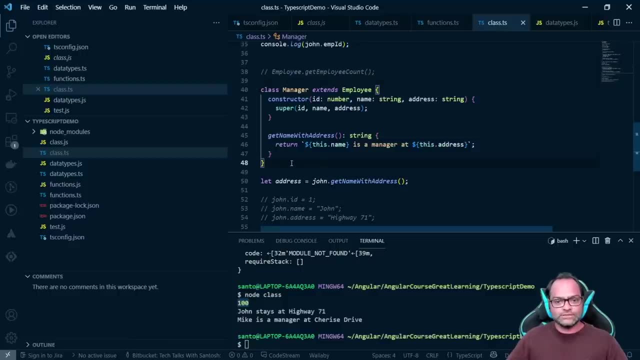 useful as well, in case we'll be using it in Angular. We'll see some examples where we use getters and setters. So this is it from the classes. We will now talk about interfaces. So interfaces are really important. I mean a lot of time you will be writing interfaces. 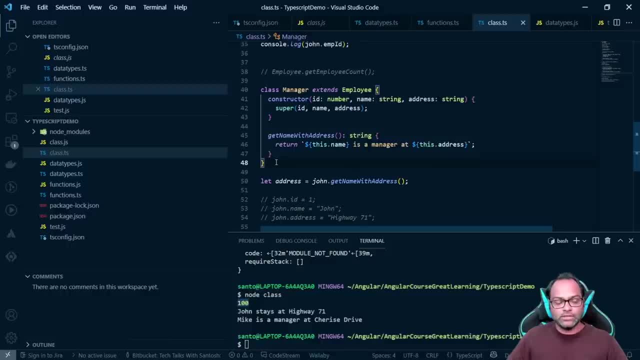 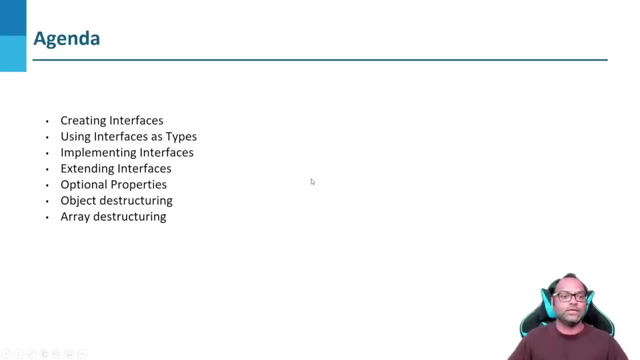 when you write a new code in Angular, or even you use it outside, Why interfaces are important. Let's see So here we will be talking about, of course, how you can create interfaces, how you can use interfaces as type, how you can implement interfaces. Yes, that's possible. 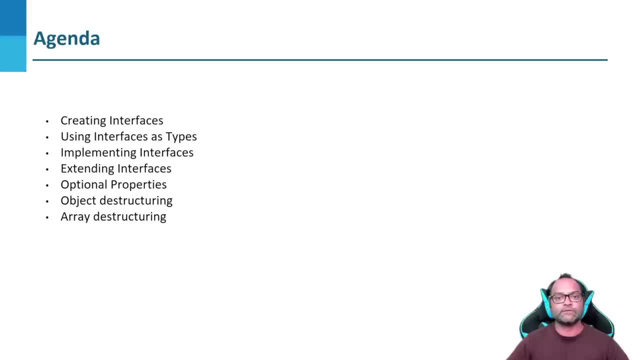 How you can extend interfaces. We will talk about optional properties with interfaces. We'll talk about object destructuring and array destructuring. That's something which is really useful. I mean, you can actually avoid a lot of unnecessary code using object and array destructuring. We'll see that. 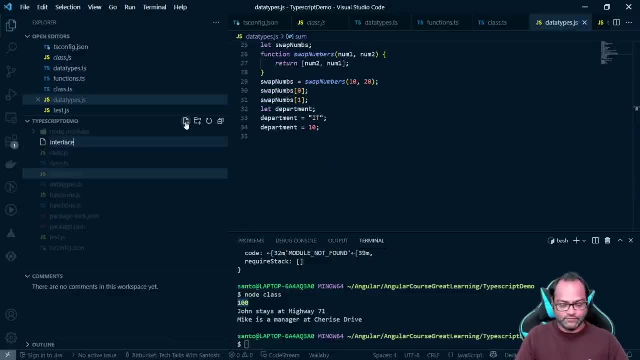 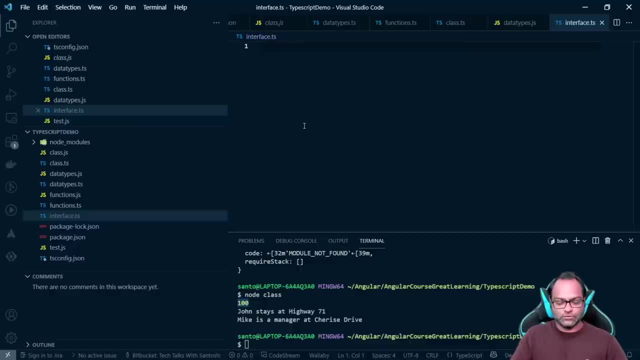 So let's create a new object. So let's create a new object. So let's create a new object. We'll see that. So let's create new file. I'll call it as interfacets. So to create an interface, you can use interface. 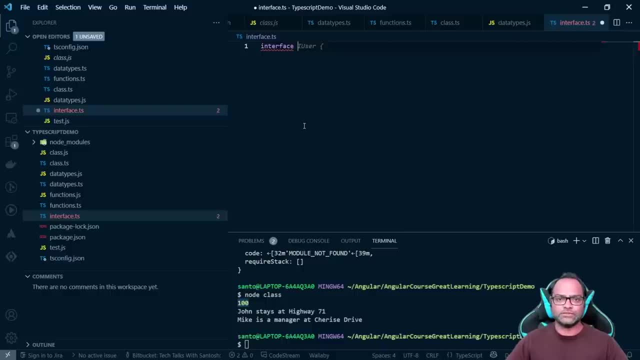 keyword and then there's a naming pattern. So a lot of developers use I before interfaces. I don't like it. I mean even Angular's documentation says don't use I. So what I can do is let's create a user interface So what a user can have So it can have a name It can have. 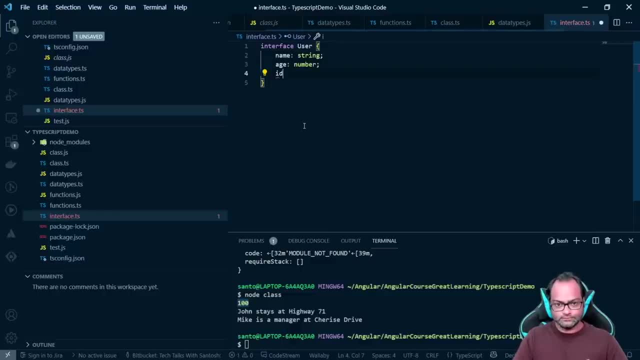 let's say, age. It can have ID And your user can have email. So these are the properties. So most of the time you will be using interfaces to create your own user-defined data type. So this is now a data type for you, So you have user. 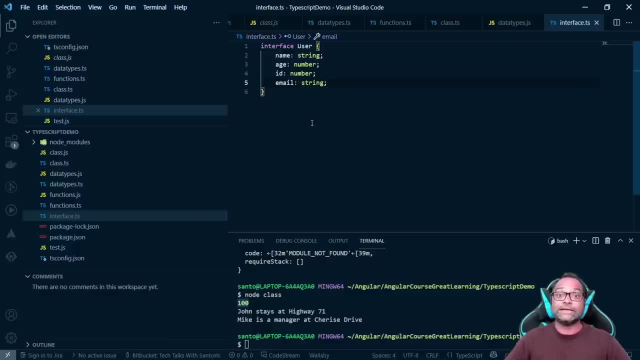 You, interfaces can also have function definition. We'll talk about what function definition is soon, But here, right now, let's talk about interfaces as your user-defined data type. So let's say you want to use complex object, So you have like name, age, ID, email. 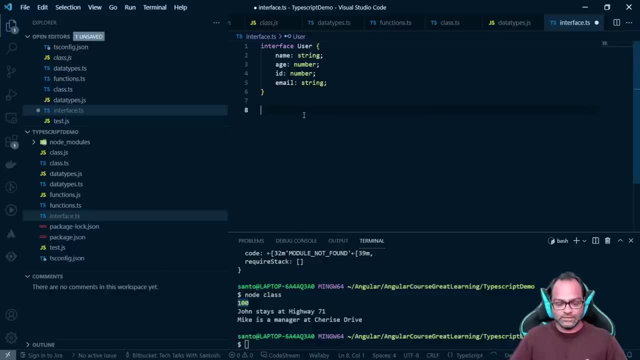 And what we generally do in JavaScript is something like this: So we create where users, for example, equals to, And then you just give all the property names, I mean, and of course in JavaScript you don't give type, So you say it has name which is like blank. 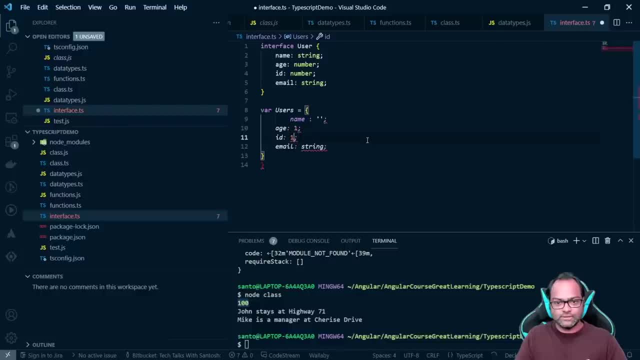 age, which is, let's say, 1.. ID has one, The default values, So, and then you can say email as something blank. This is generally. we have an habit of creating an object in JavaScript, But in TypeScript you can, rather than doing this. 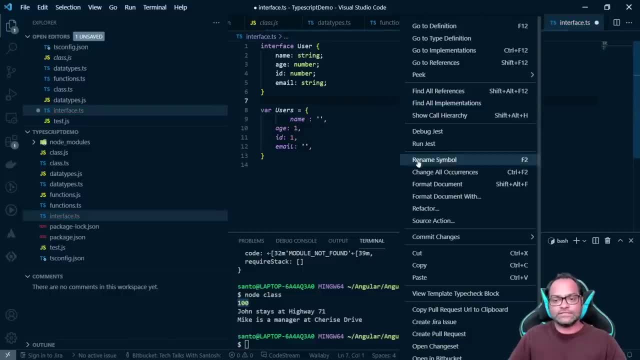 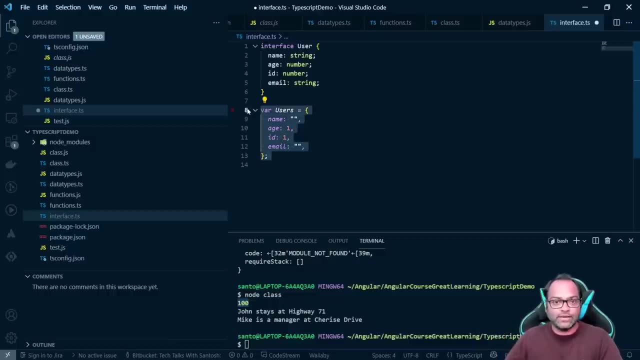 you can actually create an interface And then you can use this interface as a type, So we have type safety. That's the whole idea, right? So we can have type safety by using these values. Let's see what we can do. 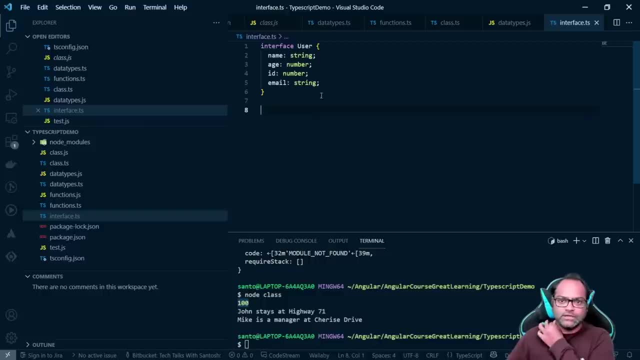 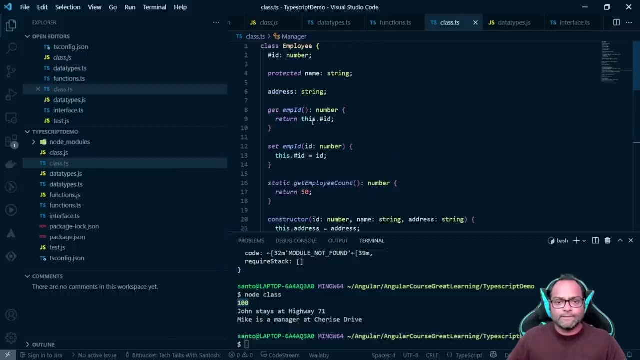 So here, remember, so we have this user here and let's try to create another interface I will talk about. let's go back to class Here: address. Do you think we can actually have a complex object as an address? Yes, we can. 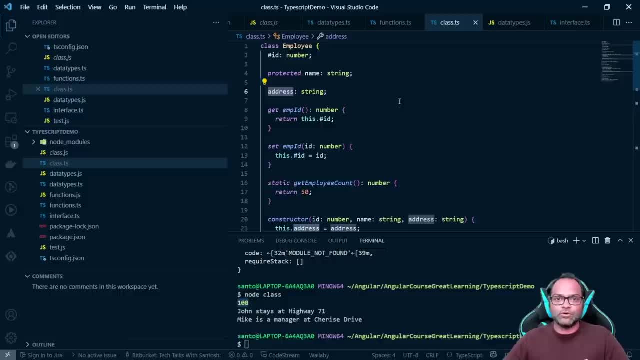 For example, we have address line one, address line two, zip code or country or city, whatever. Those are the properties which your address can have. But right now is it possible? Yes, I mean I can just go ahead and do something like we discussed. we saw right. 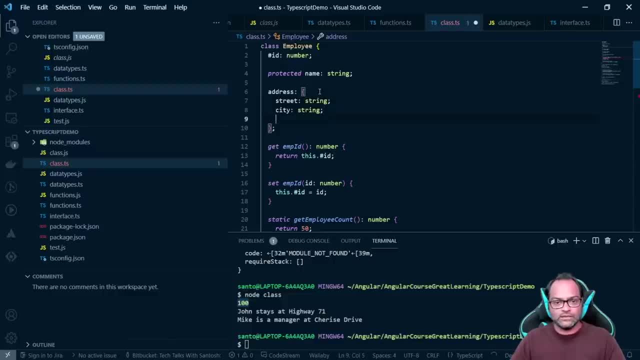 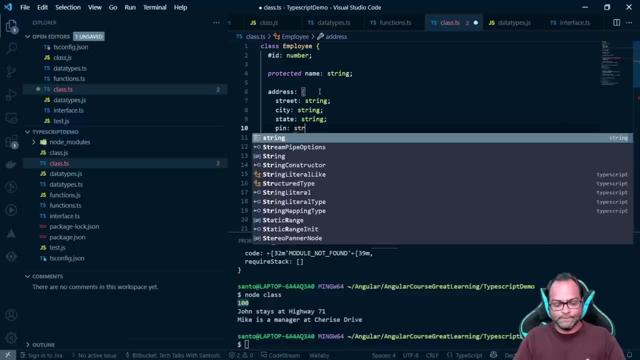 So we can have your street, I mean city. you have your state and pin, So I can say: okay, this is pin and string, So I can do something like this and you, you can see we already have address. 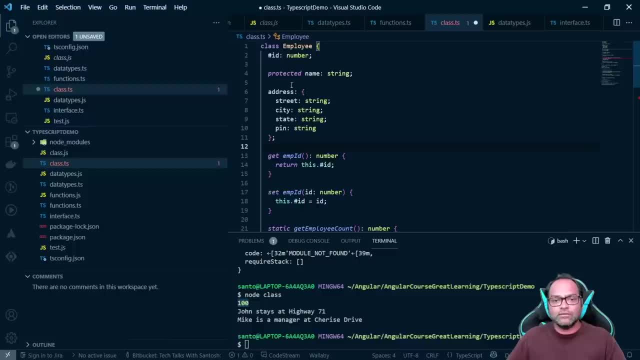 Now I can just go ahead and create an interface. We can just create a new interface. So let's say we have an interface here. We are going to use this code, right? So I can just say I want to create an interface. 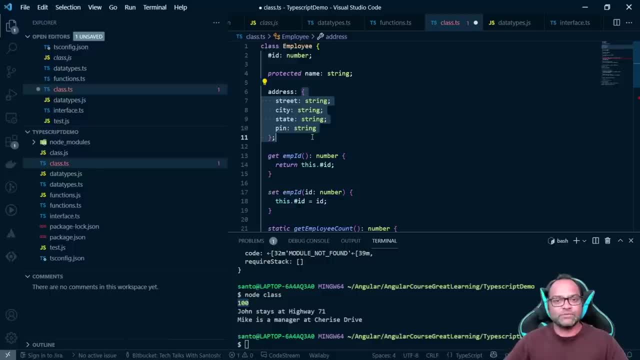 I want to create a new interface. I want to create a new interface And I can just say: I want to create a new interface And I have an error here, because this type does not match. But I mean, writing this in your class breaks the purpose. 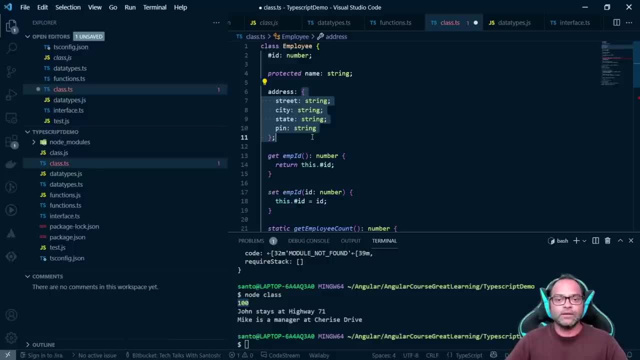 I mean, what in case I want to use this address type somewhere else, what do you? will do, Of course, copy paste the code right, Which is like, which breaks the single responsibility principle when we are talking about writing a better code. 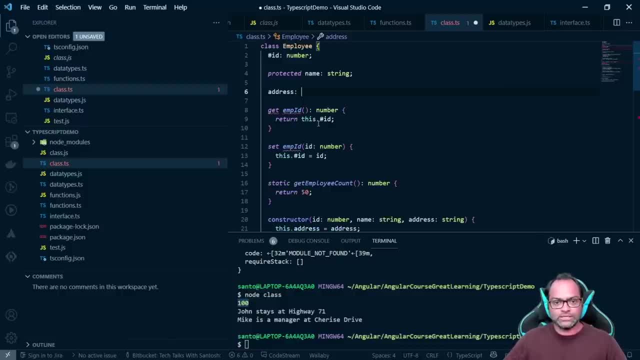 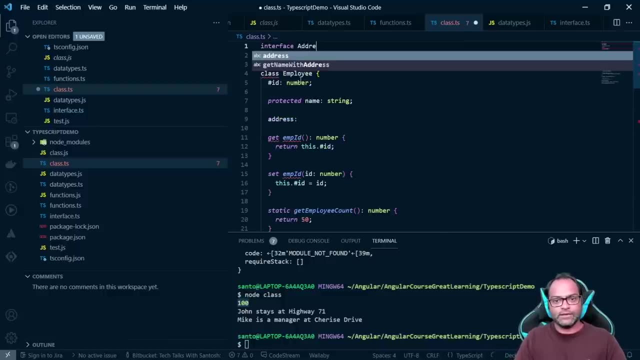 What we can do. Well, we can create an interface rather than this in this. so what they can do is: i can just create here, i'll just move on top. i can create an interface called address and, and i can have all these properties as part of this interface. now, 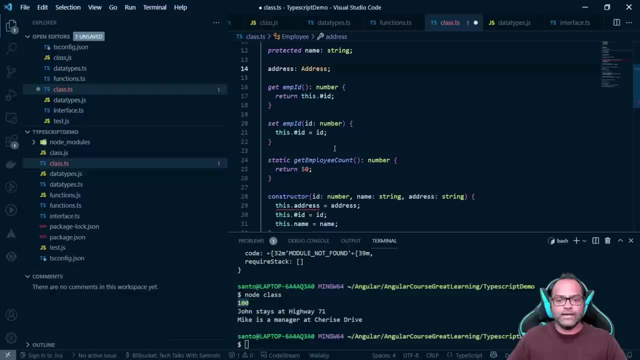 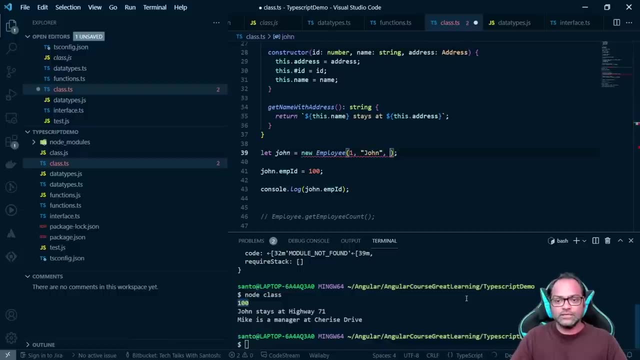 i can just say, okay, this address is type of this address. and while assigning the values, uh, here also we'll say, okay, this address is type of this address. and now, while assigning the value, you will see that we are getting intelligence to provide all the values. so you can see, it says okay, street. 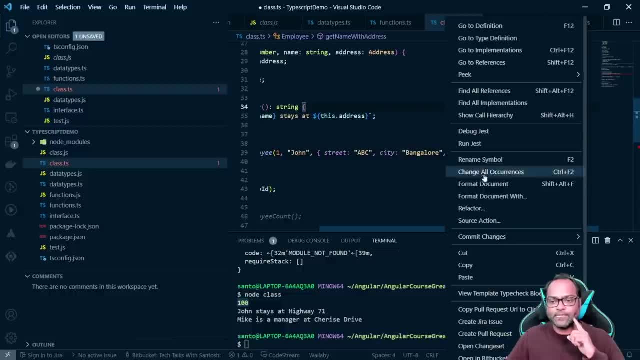 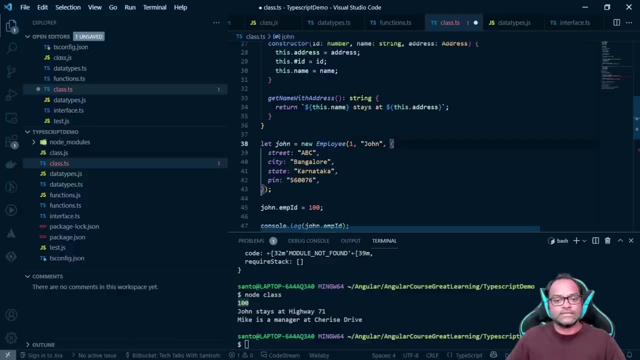 avc city, bangalore, state, karnataka, and you have your pin code. so all this are the properties which you can pass as an address and this is typed right, and so whenever your users try to actually use this particular class, they will get the intelligence. okay, these are the types which 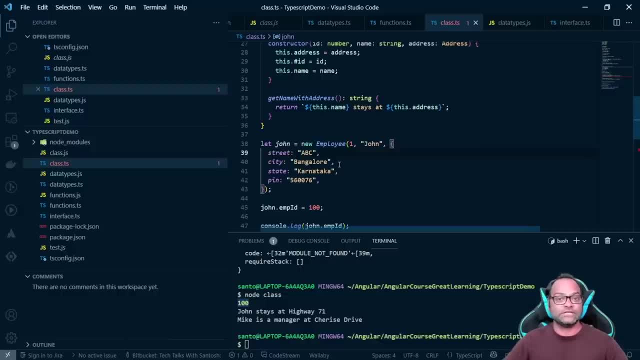 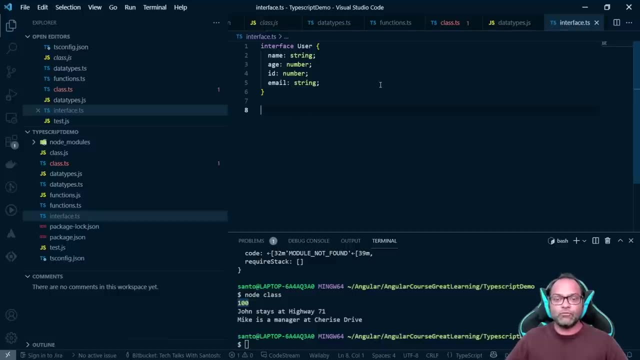 needs to be provided in case they provide something which does not work. so we can see that we are getting intelligence to provide all the values. so this is where you can actually go ahead and utilize interfaces. what in case? i want to use the interface, but i don't want all the properties to be provided. let's try to create a value here. 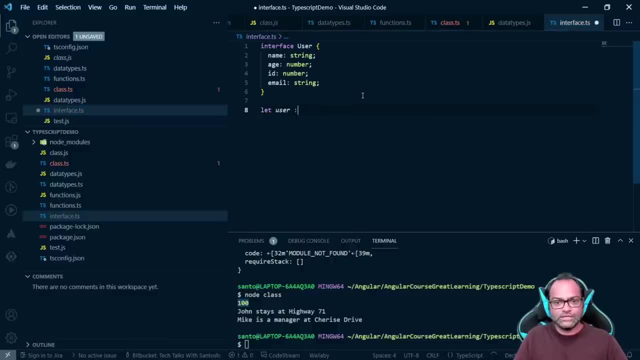 so i can select user which is type of user equals to. i mean i'll provide all the values: email. so we have john age- uh sorry, name, age, id and email. but in case i want to make age optionally, let's remove this. i don't want to pass it. what we have is an error. it says it's it's missing a property which is age, so in 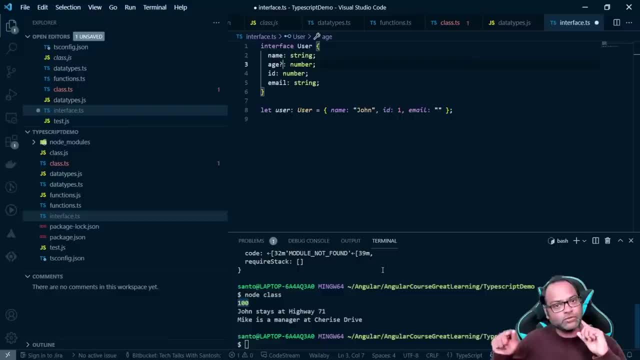 typescript, you can actually make it optional by putting a question mark in front of the property, so it it will. of course, you will get face this scenario a lot, where you want to actually make some properties optional, uh, while creating a your own type or give it a name or something like that. 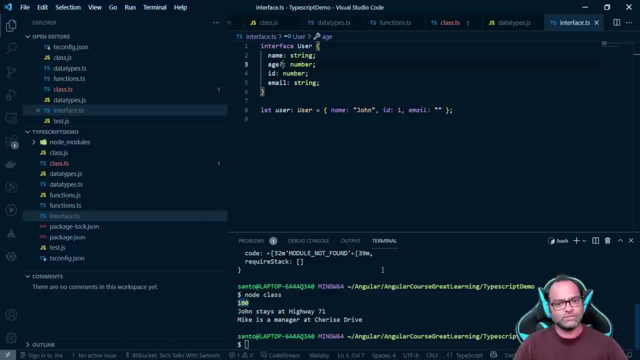 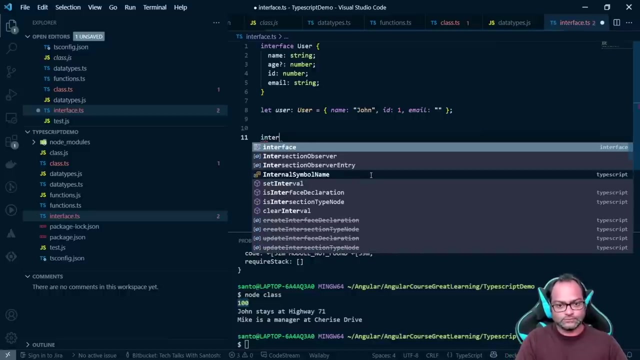 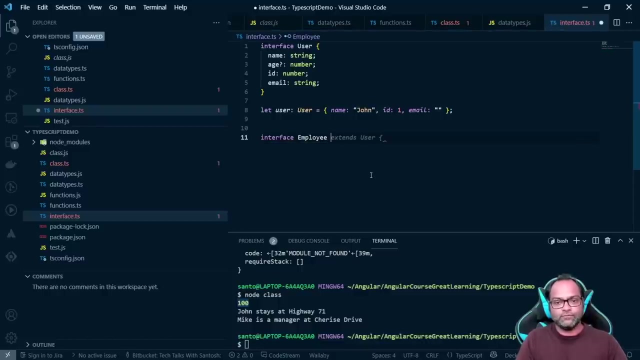 creating a while creating your interface. this is how you can do it. so just put a question mark and that's it. now let's see one more thing. you can also extend interface. you can also implement interface. so let's say: i have a new interface, i'll call it as employee and it needs to have. 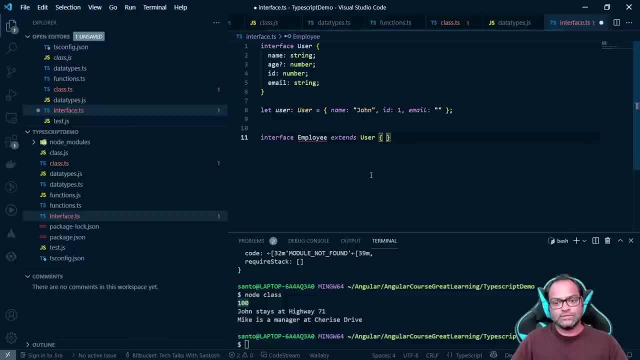 all the properties of users. so i can do is extend. so i think employee already exists. that's what employee name is: protected property name. so this was actually. we already have an employee class right, so it was just named. you cannot have actually the same name for two different. 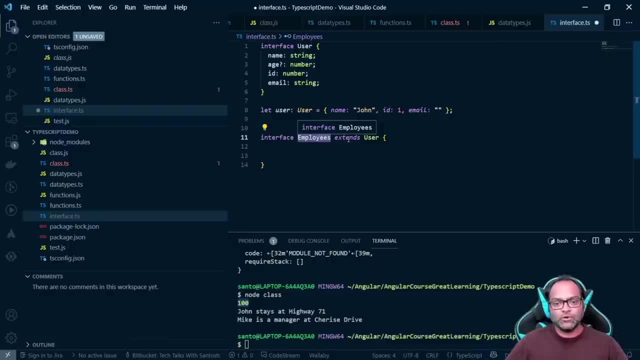 um classes and interfaces. so here we can see employees extend user. so we have all the properties which is part of user and you can also add your own. so let's say a name, age, id, email and let's say salary as extra property. so if i create a new value or create a new variable, let's say i'll 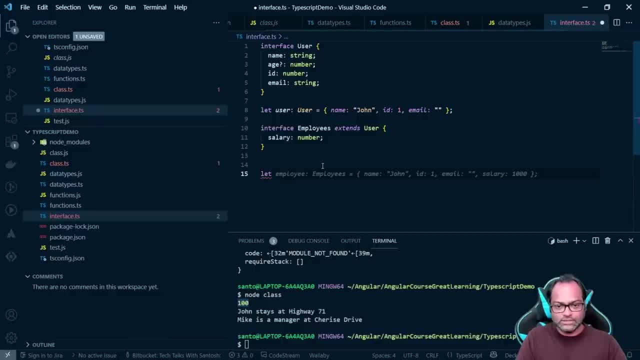 call it as. of course, let's call it as something else: let employee. okay, so i'll call it as employee, which is a type of employees. now you can see you have name, id, email, of course, age is optional, and then you have salary as well. so if i remove salary now, but you will start getting an error, that 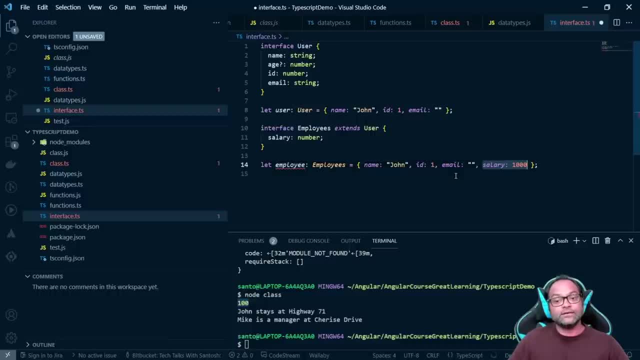 salary is missing. so this is how you can actually extend: uh, an interface. it is also possible that your interfaces can have method definition. what do you mean by that? so let's create an interface and i'll call it as login, and it has a login method which returns boolean, for example. or let's say which returns 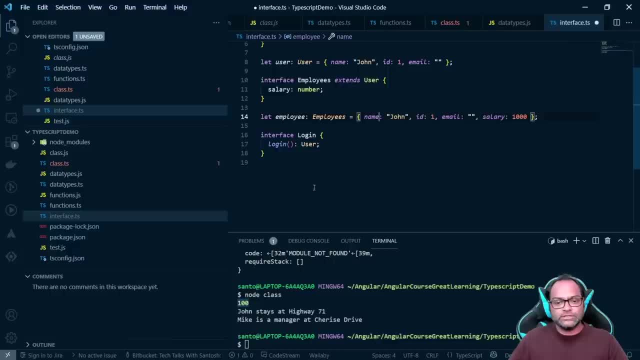 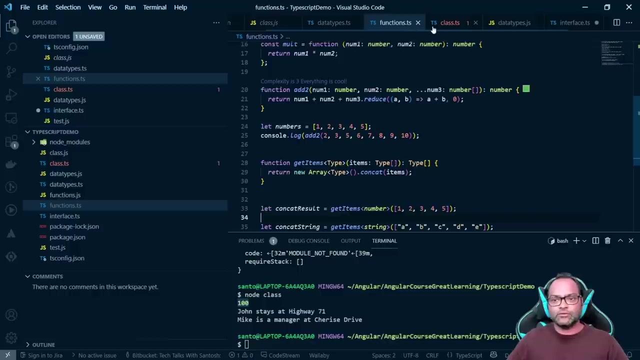 type of user. so this is method definition. you are. you are not responsible for implementing this method. who can i mean? of course, a class, so let's go back to classts. and we want to use this interface. how we can do that? this class exists in different file. this interface exists in a different file. 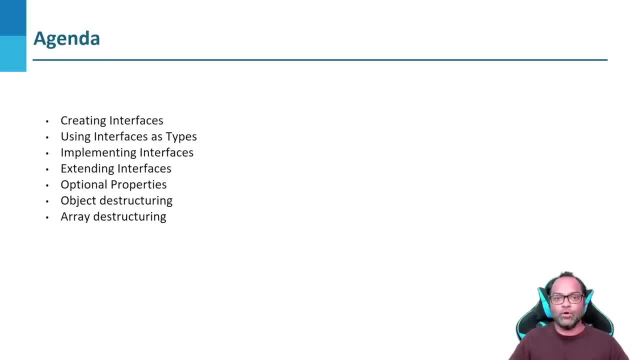 this is where we will also talk about one concept which is known as module cs, modules in type script or now available in ondesk, or set up or regardless of the says, in case we are going to write in the ofal name by a software as reflect category and placed that by using marvel, diff and uh in term undertaking. 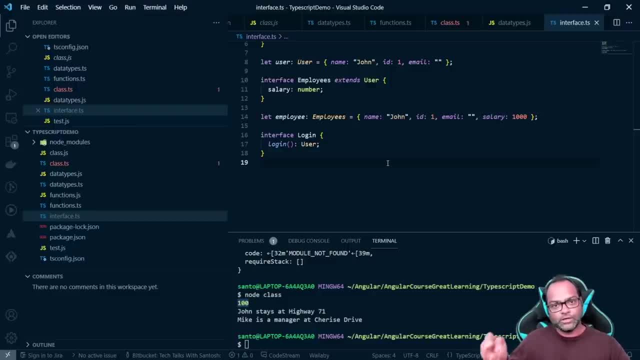 in with javascript as well. you can actually import. uh. sorry, let's not jump to the uh the terms right now, but what you can do is you can refer to some object which is which is defined in different file, into another file. how so whichever object needs to be used outside you? 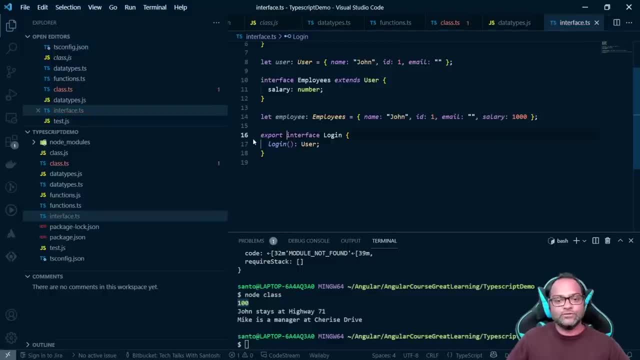 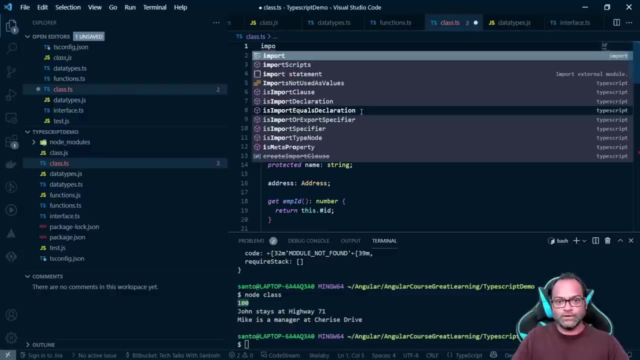 have to mark them with export keyword. once you add export keyword these, whenever it is compiled, your code knows that. okay, this particular interface can be used outside of the class. now where we want to use this particular class, what we have to do is we have to import, we have to use import. 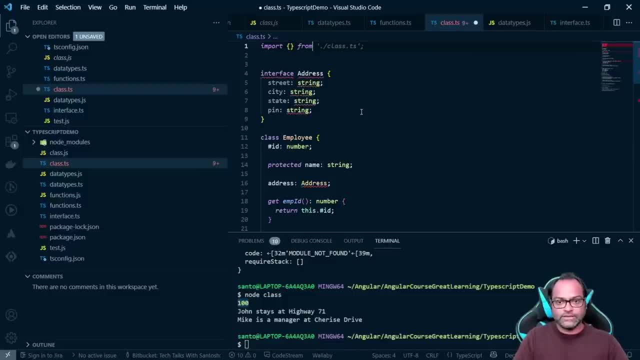 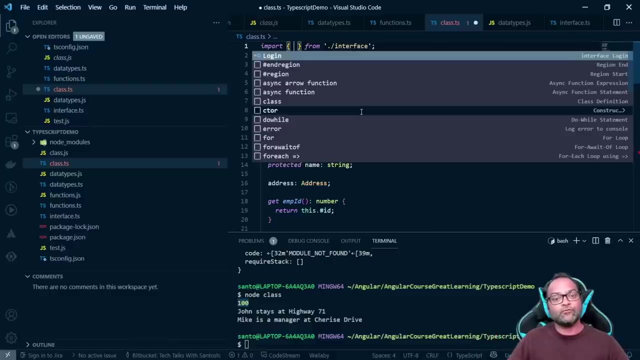 statement and then we use calibrate brackets from and give the relative path of that particular file, so that right now the relative path path is interface, don't have to give the extension. remember, i'm not using extension yet. thanks to base code, uh, you get intelligence. so once you press control spacebar you will see how. what are the things? 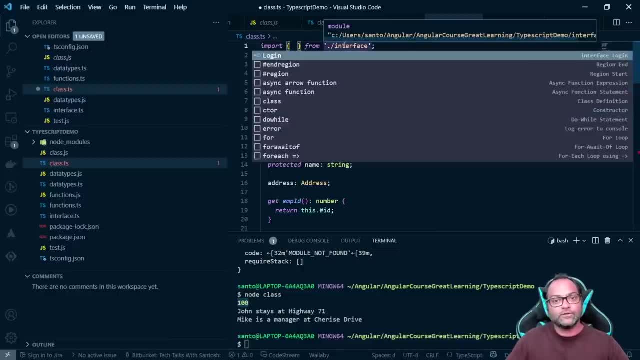 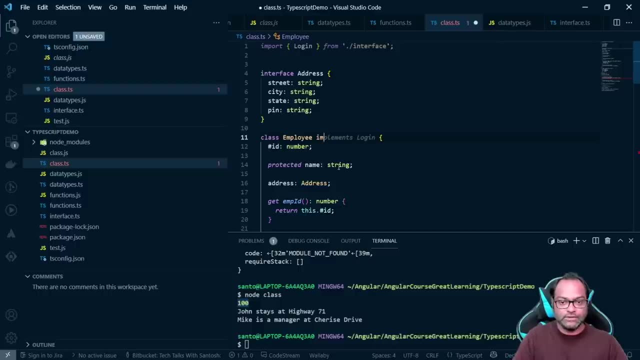 which can be used outside of this particular module, out of interface. so interface is a module and then you can use login from here. now i can just go to employee and say i will implement because i want to implement this particular function. so i can say, okay, implements login. 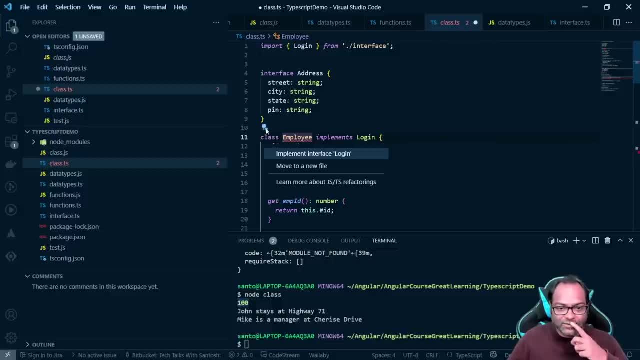 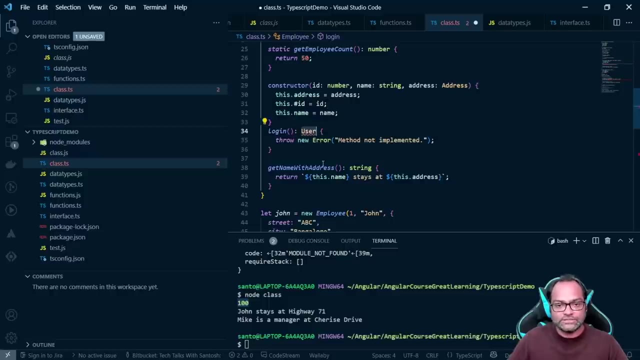 and you can see there is a of course option which says there is an alert which says you are not implementing this login- uh sorry- interface properly. so let's implement it and you can see here: so i have login and which is type of user and probably you can return a new user. 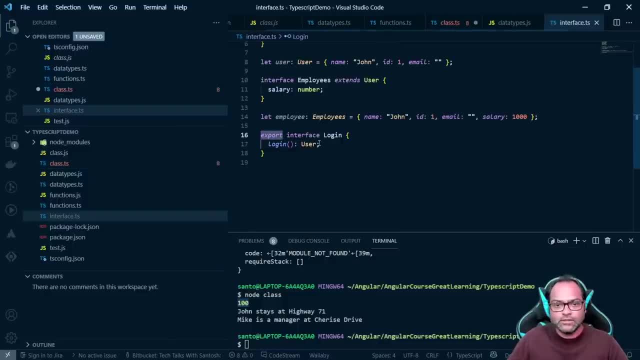 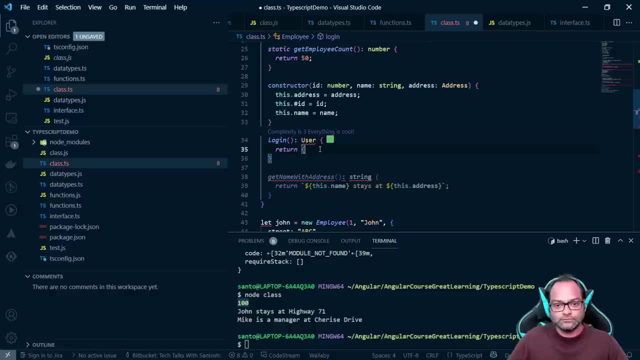 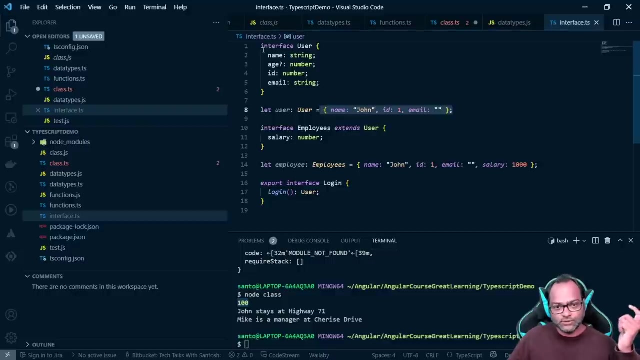 and let's copy the user from here. we already had a user defined, right, so you can just return, and okay. so here, uh, uh, uh. this is interesting. so, uh, we have said, uh, we are saying that, okay, this is the written type which is user. so what we have to do is we have to also mark user with export keyword. yes, you're. 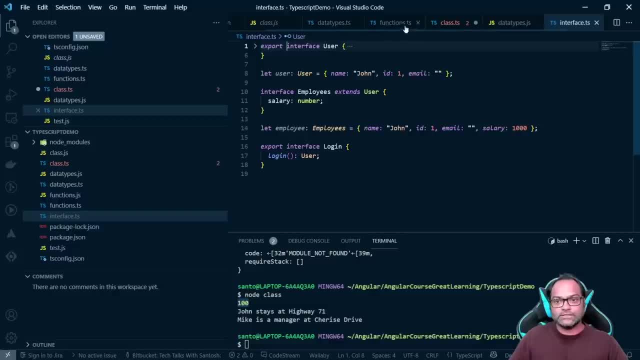 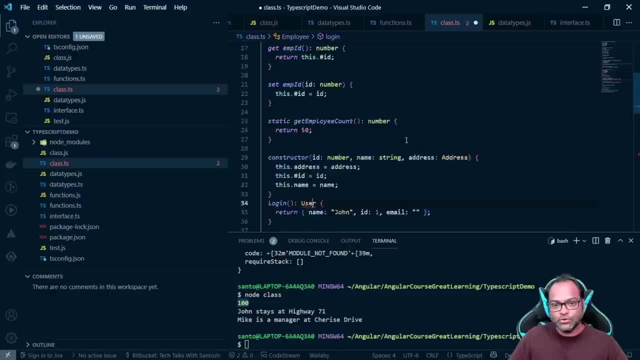 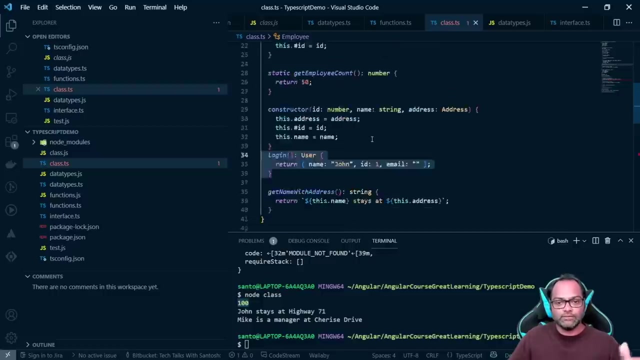 right. so we have to say, okay, export, and now i can just go ahead and use in class. so i can, if you can, please click here and you can say: add user to existing import, which is available here. and this is it. so we have implemented our login method as well. 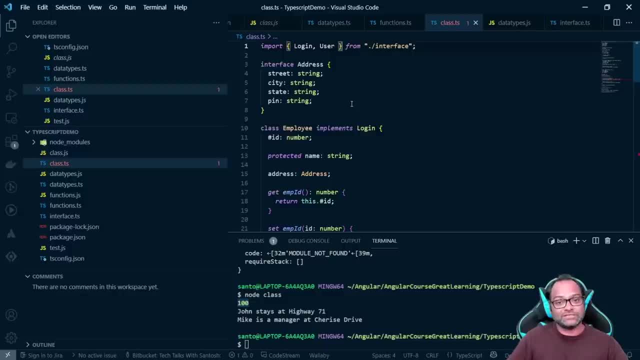 you can export in- sorry, you can import in multiple ways. so here we can see we are saying: import each object right login user. there are some other uh ways to write import statement which i generally should not use, but just in case you get across this particular syntax. 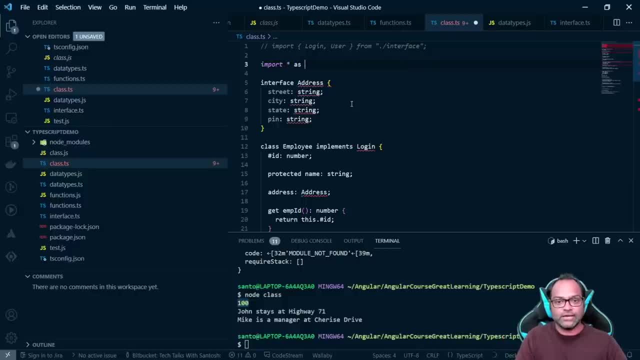 just remember that this is possible. so you can also say import star. as i'll say, this is user login from dot slash and quiz, and once you use this syntax, you have to refer everything like this: user login, dot login and here as well, user login, dot. use it. so that's, that's the only syntax. so it's a. it's an. 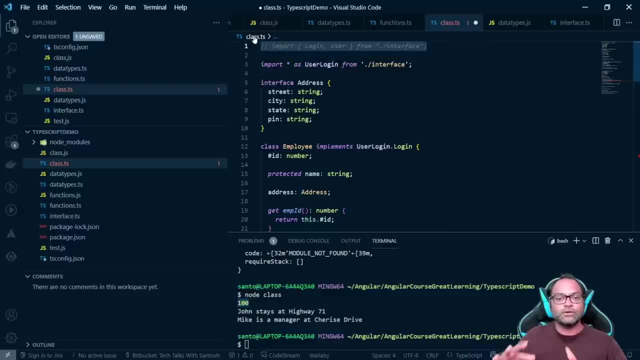 alias. we are saying, okay, whatever this particular module gives to me, uh, use it as alias user, use user login as an alias, and then i can access every object by using dot. so don't use this. i mean, this is something which you should not just use whatever you need and that's it. so this is how you can also. 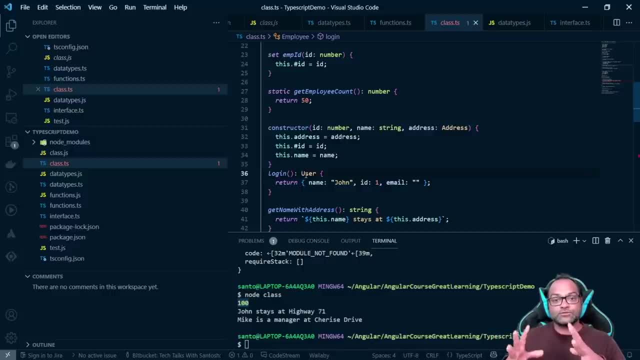 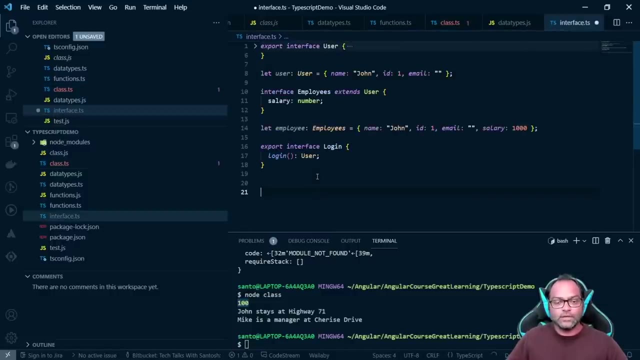 import and export, which is known as es modules, and this is also you can, how you can use interfaces. now we will talk about object destructuring and edit destruction. let's see, so let's say we have a function which returns the user information, right? so let's, rather than function, let's have this object. so you have this user object and 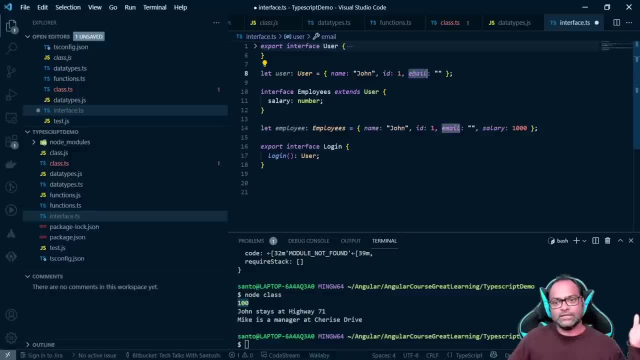 what we need is: i need to access name and email. that's it. i just need two properties, how you generally do that. so this is the way. so you will, of course, create this user object and then you can say user dot name. that's it. i want to access it so i can say username and user dot email. 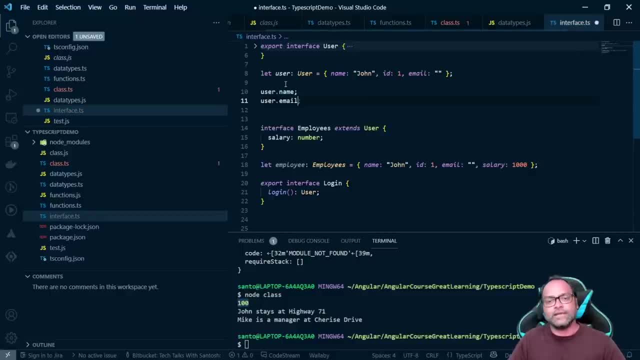 right. so this is how you will generally access all the all the objects. but in case we actually can write this in a single line of code, yes, that's possible. so here, uh, what we can do is we can do something like this. i can say: user comma, email. 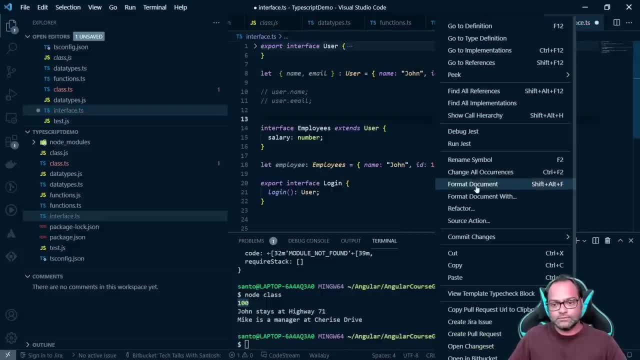 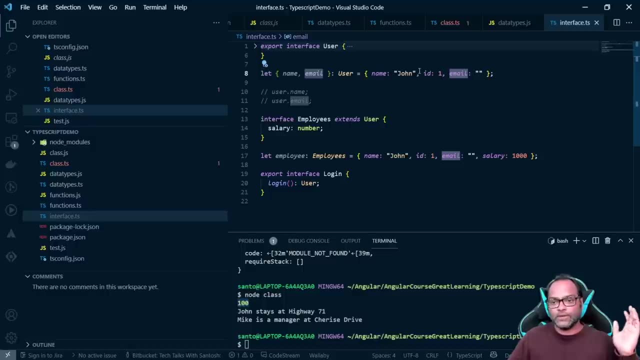 sorry name. so we i can say, uh, this is known as object destructuring, so we can just access name and email above out of these three properties. i don't want to read id. that's absolutely fine, you can also rename it, for example. i just don't want to. 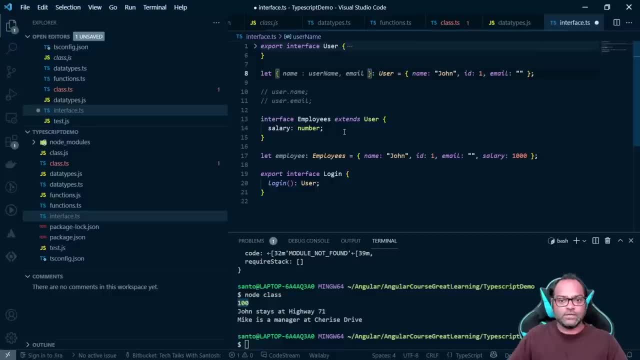 use it as name. i want to use it as user name. i mean i want to access this name property, but not as name property. i mean i want to rename it as a username. so what you can do is name colon whatever new property name you want and that's it right. and for example, email. also, i don't want to name it as. 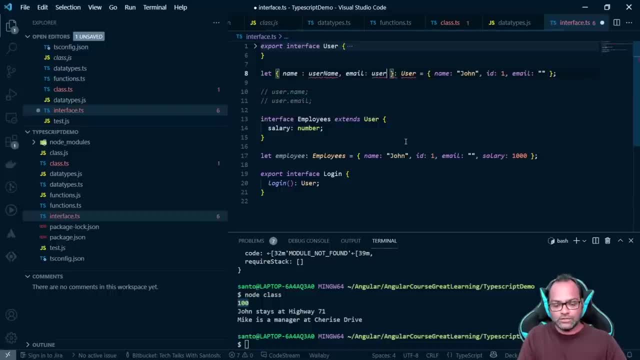 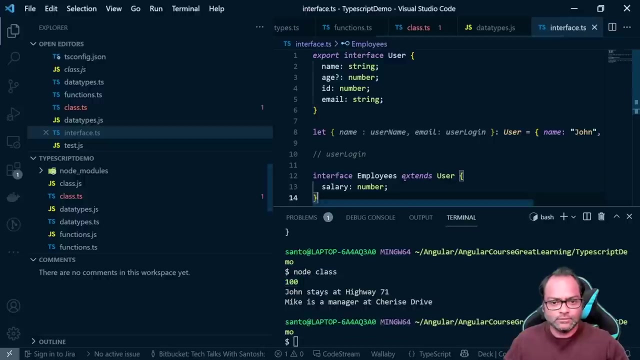 email. probably I want is user login, right. so now, if you see here next line, I can just go ahead and use user login as a, as an property that's available. so this is object destructuring, which we can generally use. let's talk about. let's talk about array destructuring now. so 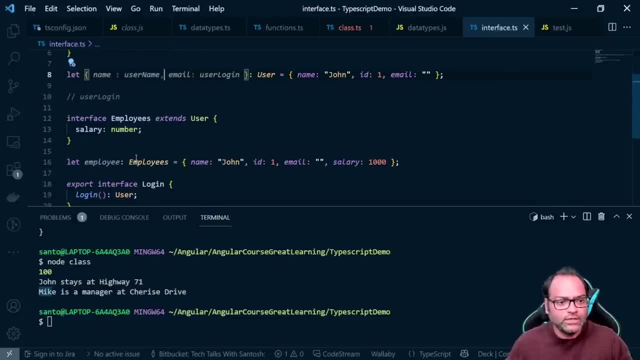 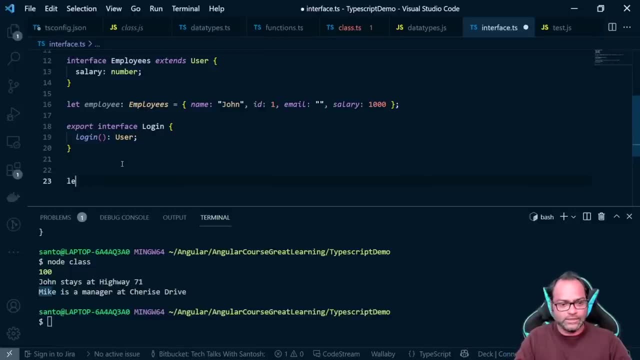 we have this object destructuring and to create or to learn about array destructuring, let's create an array first, so I'll create let users, which is type of user, and n. so, as mentioned, you can use both syntax array with like brackets, which is a generic 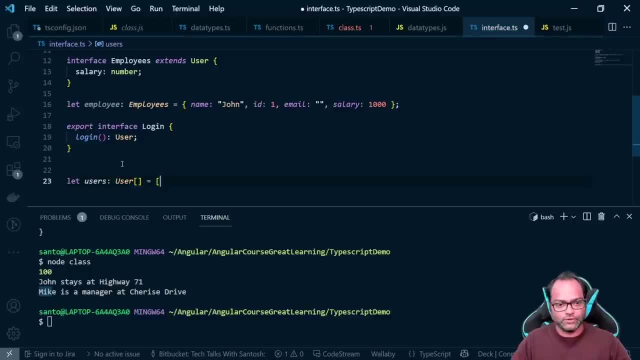 syntax, or this syntax, and let's create few records. so we'll say name, you know email, let's copy from here: I think we have this and let's format this and that. let's add one more, few more records. so I'll say to this is so I can say one, this is two and this is three. I'll change the id and john: one, two now to 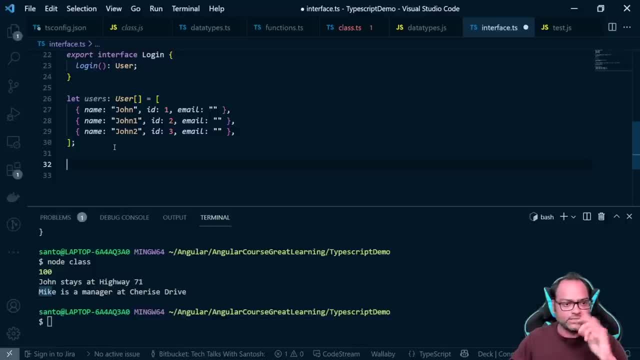 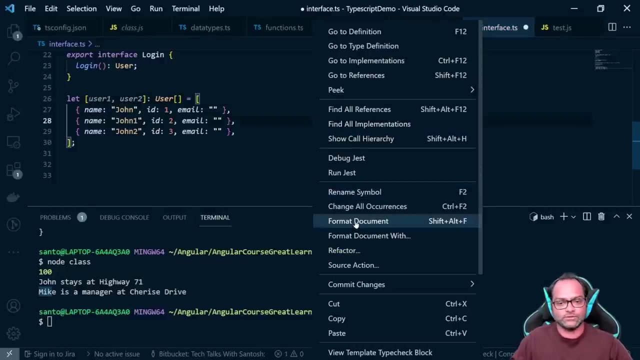 learn about array destructuring. let's say I want to access the user one and I want to do that, so I can say user one and user two. how we can do that, any idea? so of course we need array syntax. so I will say box and then I can say user one, command user two, and this is it so. 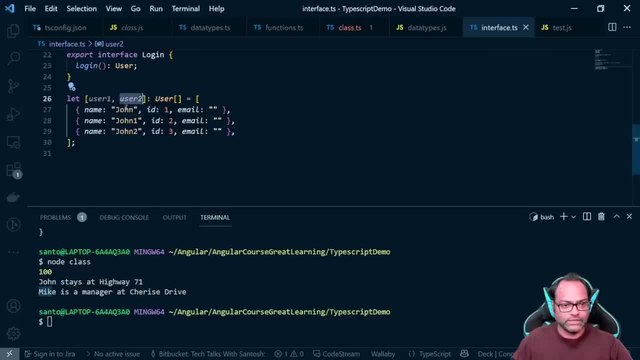 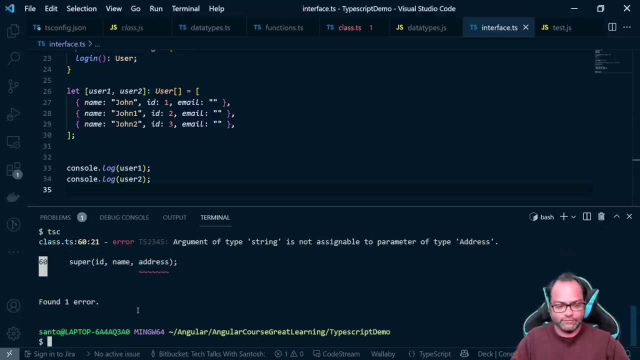 you will get the first record in this, second record in this let's. let's try to write console dot log and see if what we are talking is correct. so I'll say console log, user two, and then I'll two, so it's a dsc and then we will run node. this is interface. so i'll say: okay, there is some typing. 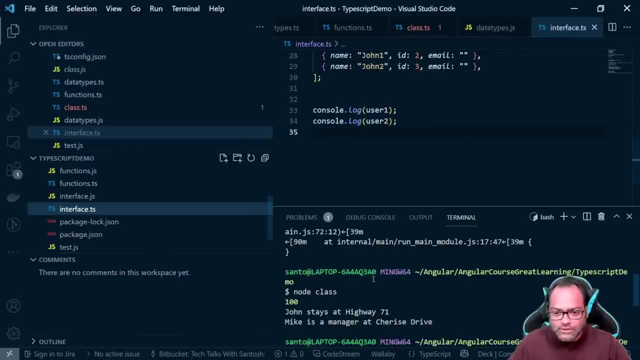 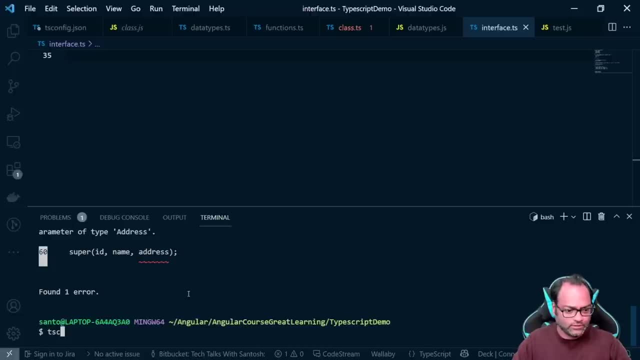 issue which we changed. it's okay, so anyways, it's, it's, the files will anyways compile. so not a problem. not a problem here. so it's a node interface, so you can see, you have like first record here, second record here, and you can also have all the values, the rest of the values, like 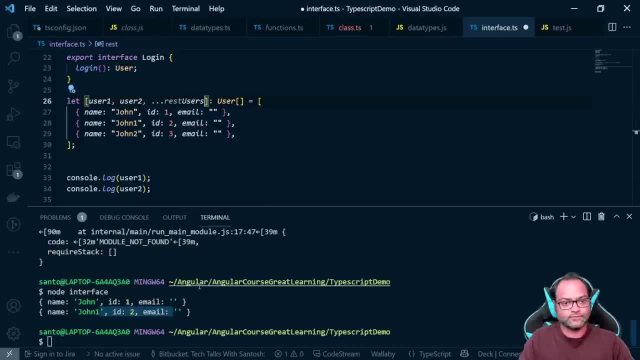 this. you can say you rest users. so let's say: if i have a few more records right, so let's say, look at this is user john v and id is four. and let's do consolelog user three, also consolelog rest users. so let's use tsc again to compile the files and then we will use node. 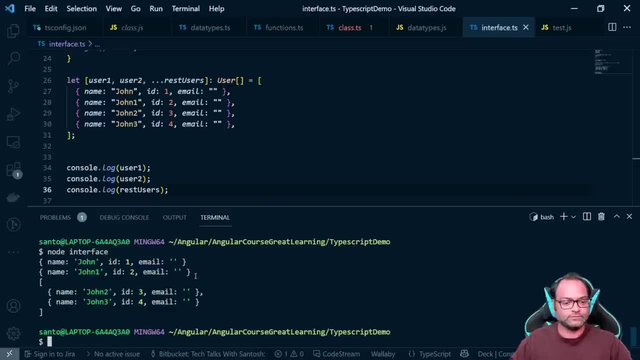 and you can see: uh rest of the values are available as part of this particular array and you can see these are objects. you don't have to actually go ahead and get it as object array and then you have to access the values. it's not so. you don't have to do index. 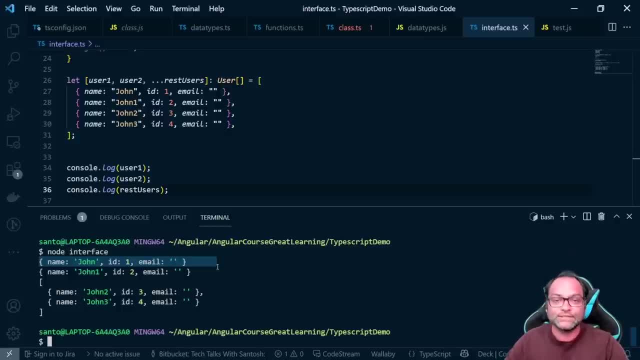 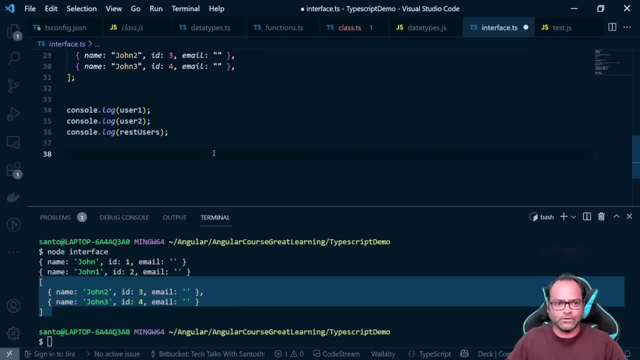 of zero index of one. that's something which we don't have to, in case you are using this array destructuring syntax and you can get rest of the values like this: all the rest users. so this is really handy in case you are working with arrays and there are a few more functions. uh, let's few. uh, let's talk about few. 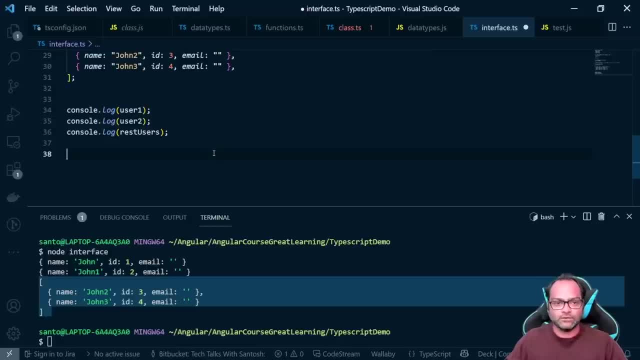 uh, let's say, if i want to filter, uh, a value like, so i can say, uh, let's say it is equals to this users. uh, yeah, let's use the rest users, and here you can use filter, for example, and then you can say: user id is greater than two. so what are the? 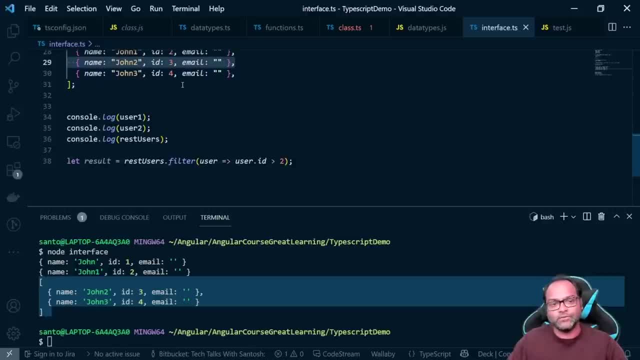 values, which is this: uh, three and four. sorry, uh, we only have three and four in rest users, so i can say, okay, greater than three. so i i will get one one record with this id four. i think we we already discussed about few array methods, so let's not talk. let's not, uh, go ahead and talk about them. 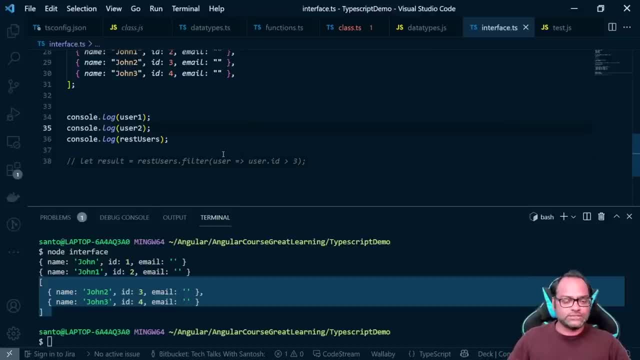 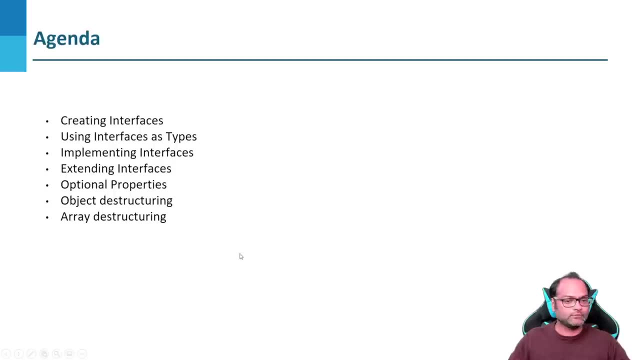 so that's it, that's fine, and uh, this is this is it about. yeah, so this is it about, uh, interfaces. one more thing: uh, before we move back, so we need to talk about decorators, uh, but before that, before we move into decorators, one more thing which we 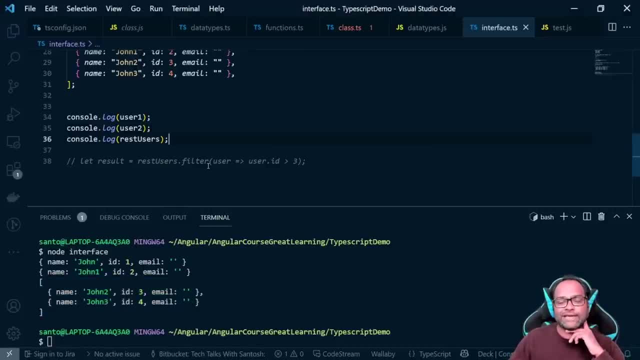 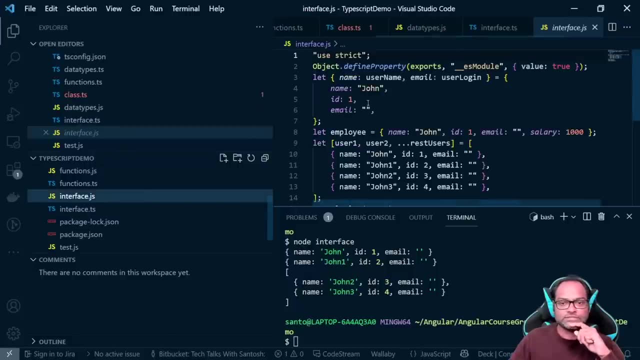 uh, let's talk about so interfaces actually does not exist in javascript, so let's see the output. so we have this user interface which is created right, so let's go ahead and see interfacejs. you will not find that particular interface which is created right, so let's go ahead and see interfacejs. 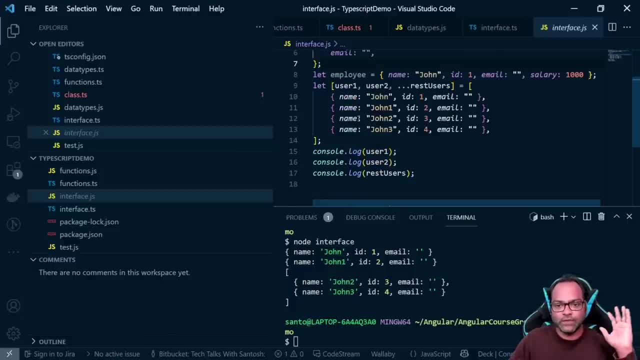 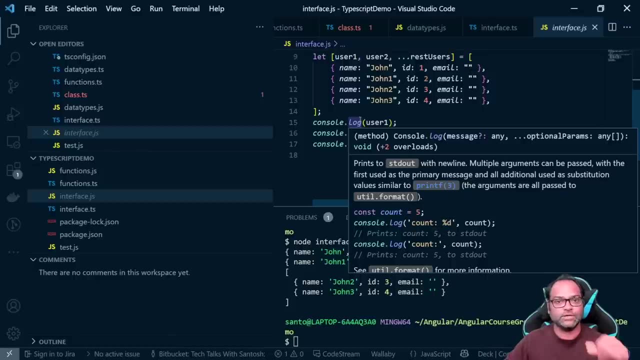 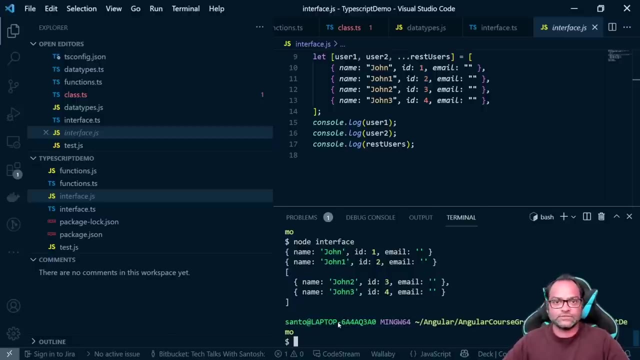 anywhere. so, uh, remember at runtime all the interface, i mean, once you compile, uh, your code, all the interfaces will be removed, they won't be part of your production bundle. so you have to decide whether you want to use interfaces or classes. this is generally which people do ask. 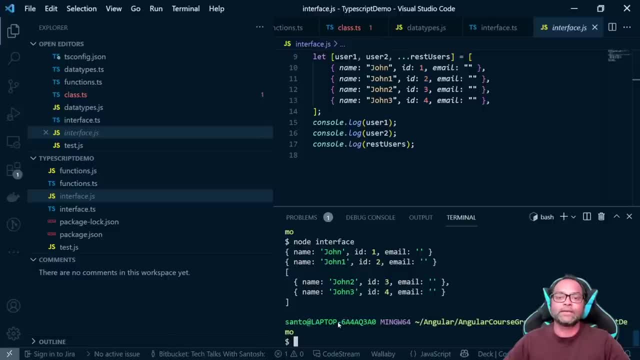 that when to use interfaces or when to use classes, in case you want to actually retain the type by like, once you create the product, build, go ahead and use classes, because generally used in like back-end programming. so if you are creating your apis, it is preferred that. 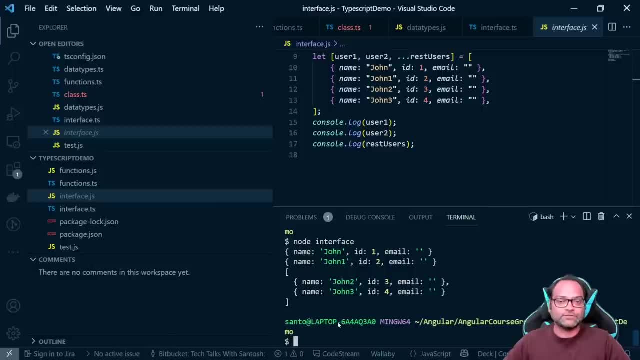 you should use classes for written types, not interfaces. for example, if you uh come across nestjs or you use expressjs, where you have to actually give some, take some input, you cannot use interfaces there because of course, once you create or build, the types are gone so you can use. 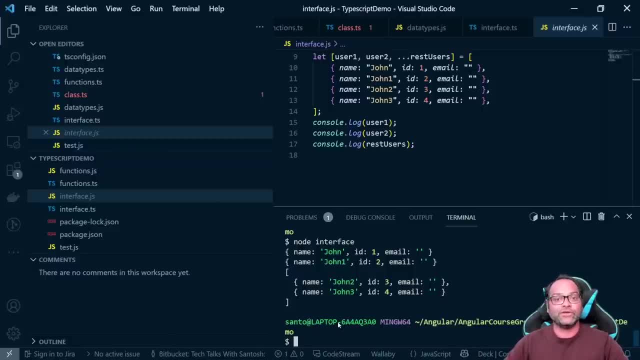 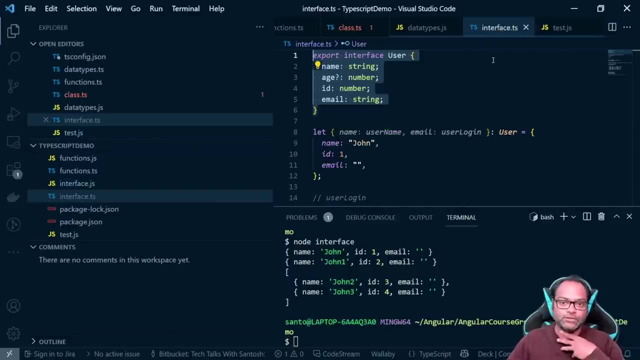 classes, and then you can retain the type and you can also verify if you are using interfaces or using uh, if you are getting the correct information or not. so just keep it in mind. so this is something which, um, which is really confusing for someone who is coming from java or dot in background. 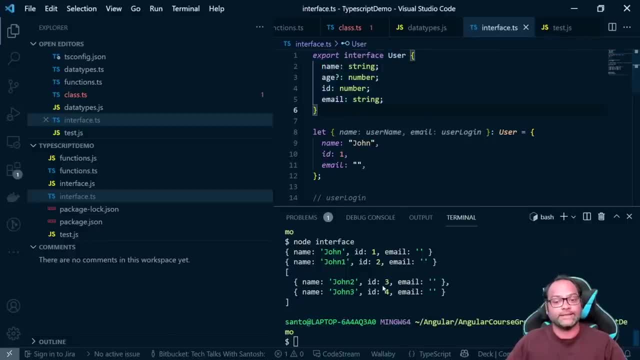 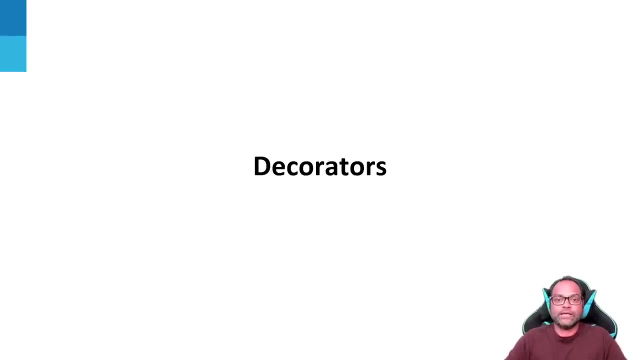 but yeah, this interfaces does not exist really inside uh timescript, assuming javascript. so decorators are one experimental feature which is available in typescript and it is not going to go anywhere because a lot of users, a lot of frameworks, libraries already use decorators a lot. it was initially. 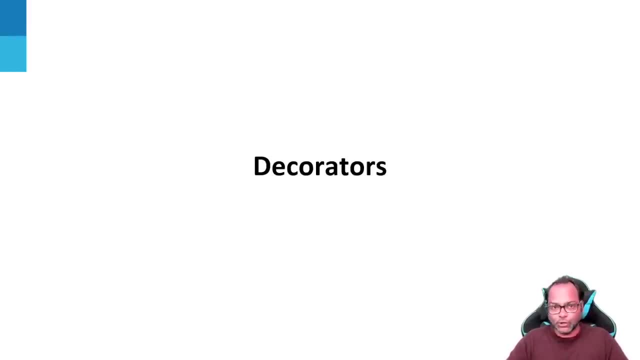 suggested as part of javascript, but it was later dropped, so that's how they still exist inside typescript. they can be applied on like: um, what, what is a decorator? so it's, it's like: uh, you can also. you can actually go ahead and modify the behavior of your class or method or a property at runtime by using decorator. 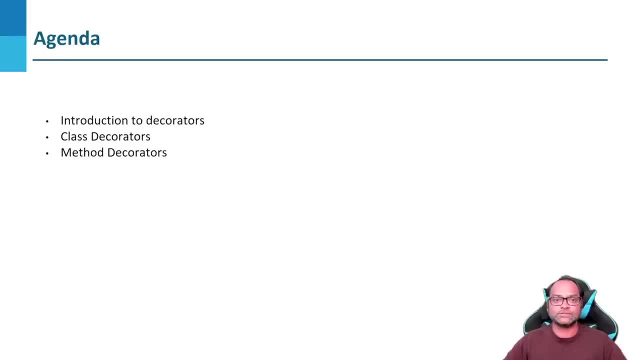 so are we going to write a decorator? the answer is, most of the time, no. that is, uh, some advanced code where you may need it. why we are talking about decorator here? because it is used internally by angular and you will come across multiple decorators when writing your angular code. so 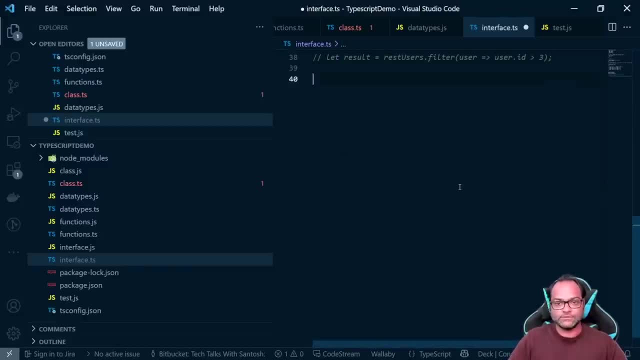 let me go to codebase, so some examples which we will see. here are some examples which we will see is, for example, class, let's say component, and you will come across, let's say, a decorator called component. so what, this particular component? so generally, whenever you see something on top of class, 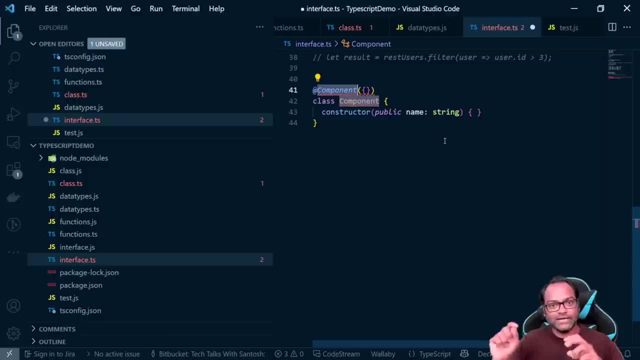 or property or a method, you will use the decorator and then you will see that it is a decorator in the form of a decorator. so in case of the example you want to write a decorator, you will use the decorator, with starting with at the rate and having some curly brackets and some properties. those are 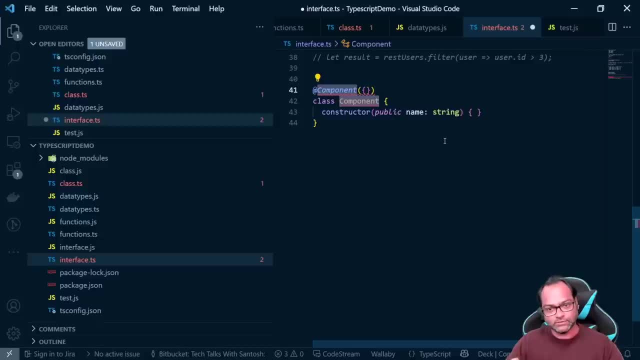 decorators so it can be change the behavior of your class at runtime once they are executed. we will not be writing our own, as we said uh, we will be using the one provided by angular. that's why that's the reason we are talking about uh decorators here. you can actually write your own. 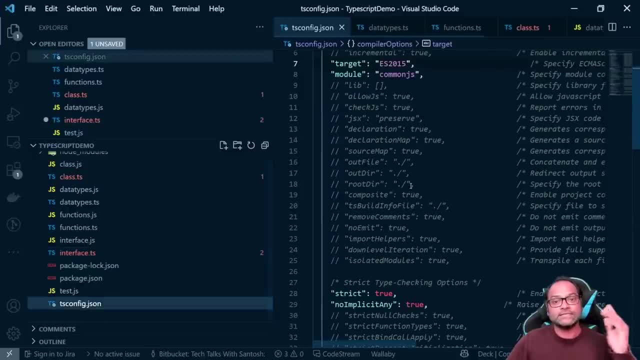 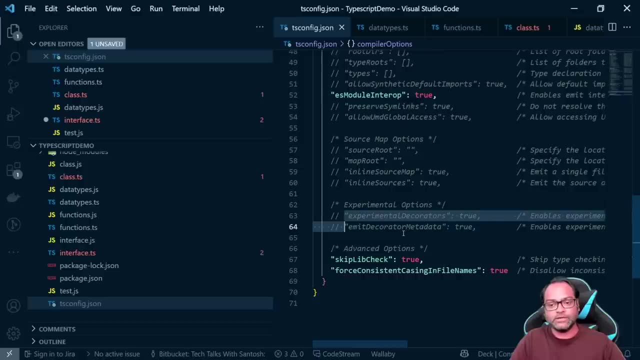 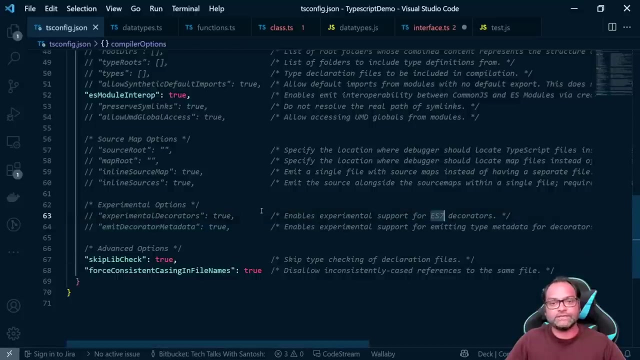 as you use case, you probably will never come across that. as i said, these are experimental features. so there are two flags which is used: uh, this one, experimental decorators and experimental decorator metadata. this needs to be enabled. so here you can say: okay, enable this experimental support for es7 decorators. this needs to be enabled here, in case you are writing your own. 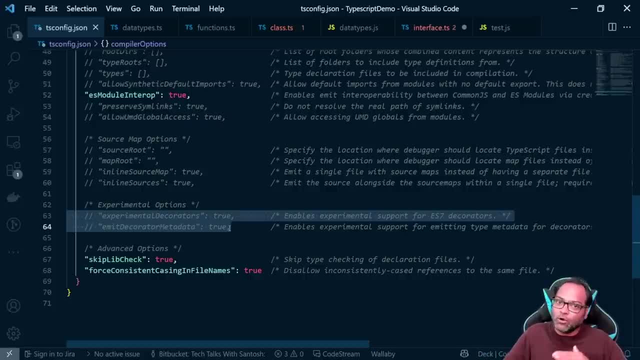 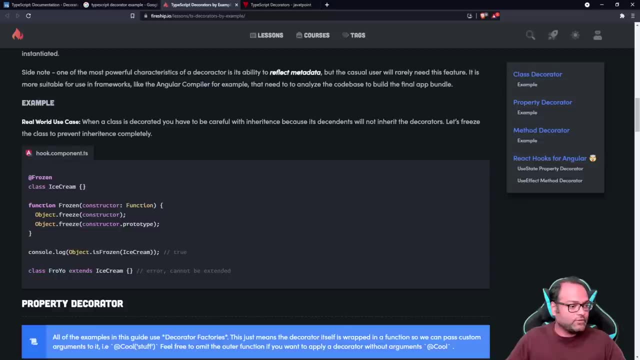 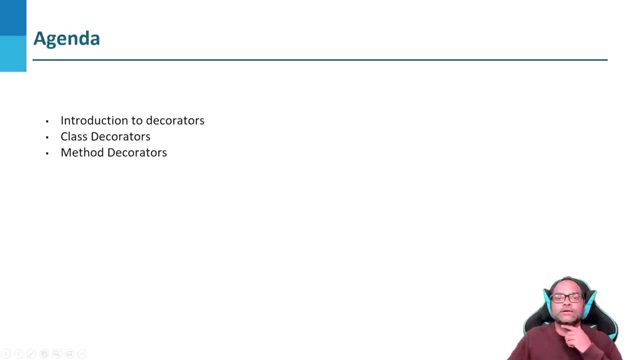 typescript code outside of angular, but inside angular these are already enabled, so you don't have to do that. so this is it from. so this is it from decorators. we will not go, we are not going to go into much detail. let's talk about es module. we already saw the example while working with interfaces and 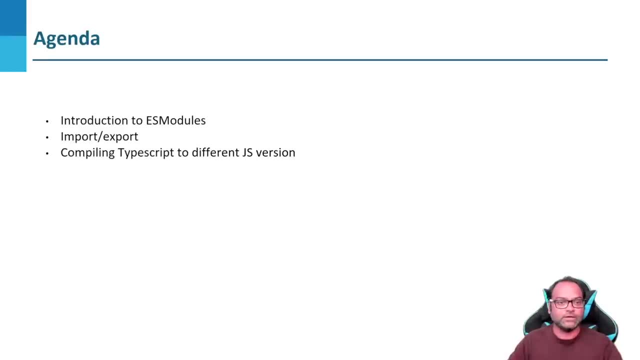 classes. you remember import and export keyword. that's what we- this is what es module is all about. and let's see, uh, we also went through. actually, this is also. We also went through TypeScript to a different version. You remember we changed the target to ES5 and ES2015. 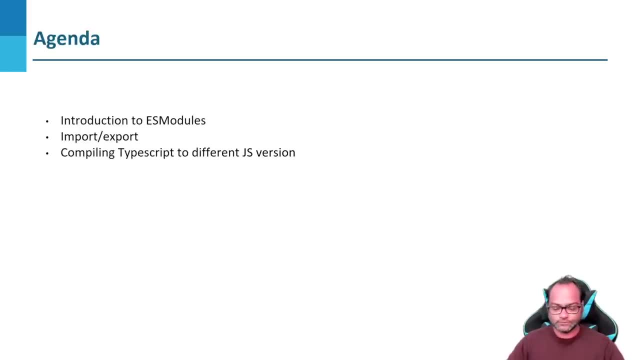 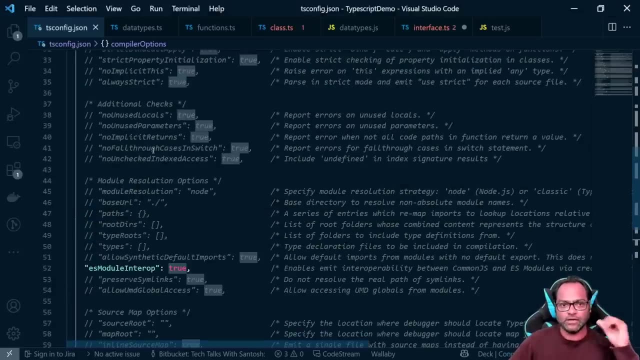 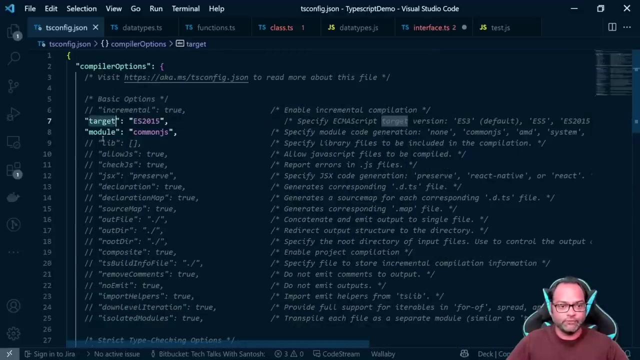 You can change it to whatever version you want. And let's see some properties of this tsconfigjson file, And then we will end with our TypeScript section and we will start with the Angular section. So here, as I said, we already went through target and module. 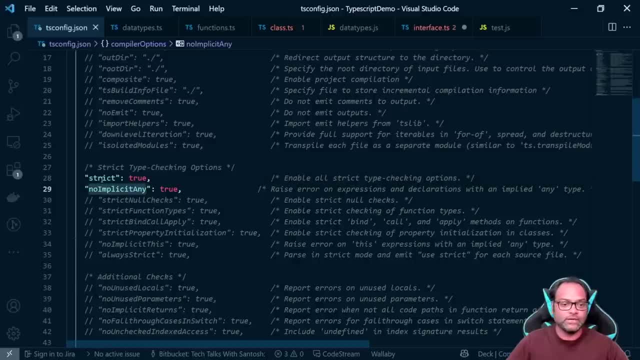 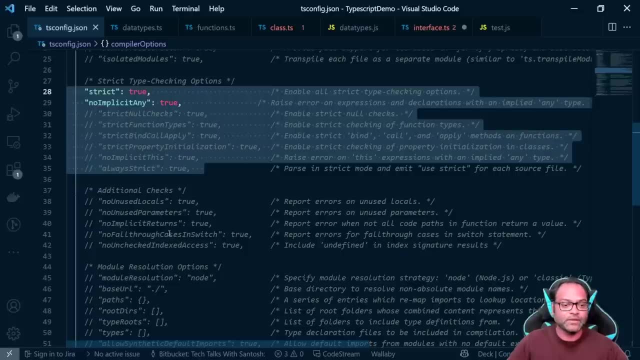 We saw strict, no implicit any. just enable it as well. But if you see, say strict, true, you have enabled all the strict flags here. You don't have to actually enable one by one. Apart from that, you can use some of the properties. 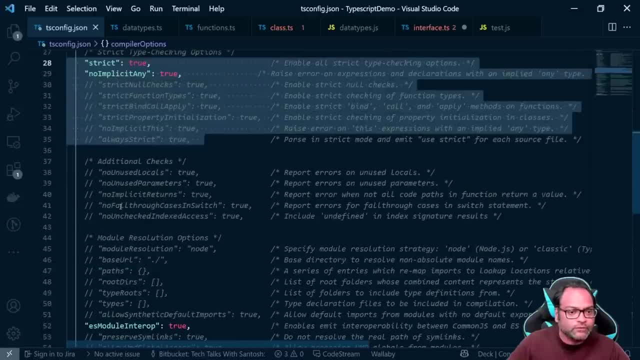 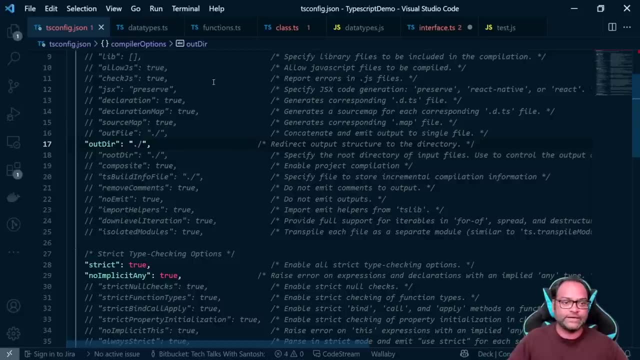 for example, here, output, output, output. Can we see output here? Yeah, out here. For example, let's say, I want my all output which is generated right now. let's see. So, if you notice this, this file is not saved somehow. 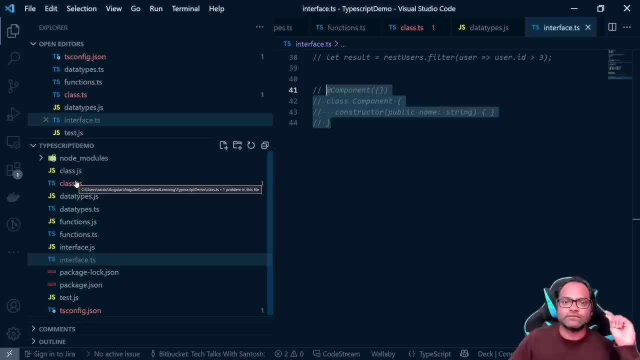 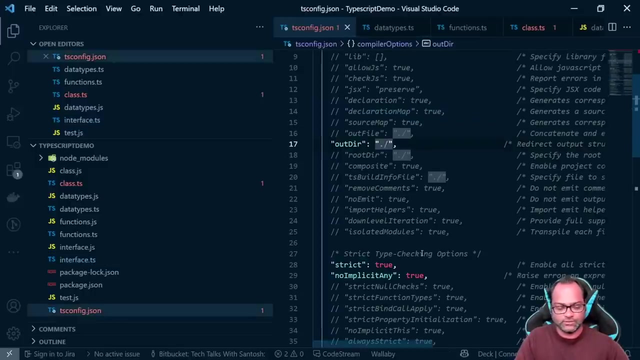 If you notice, right now all the JS files are just created next to our TS file. What in case you have a lot of files, It will make your life really tedious to actually go ahead and figure out which file is your output. So, using root DIR, I can just say: 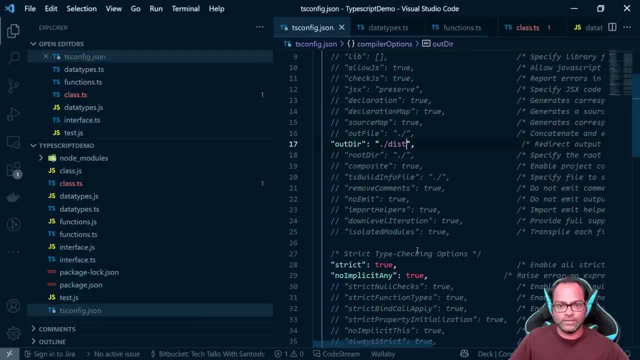 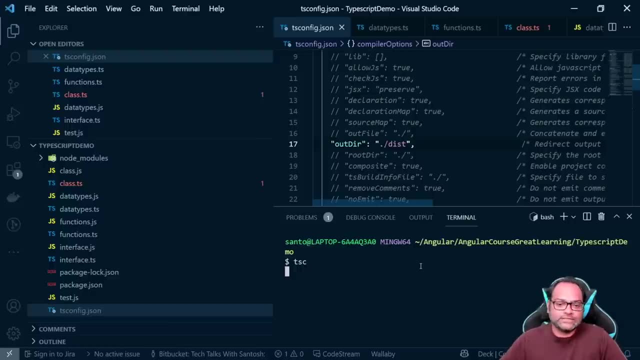 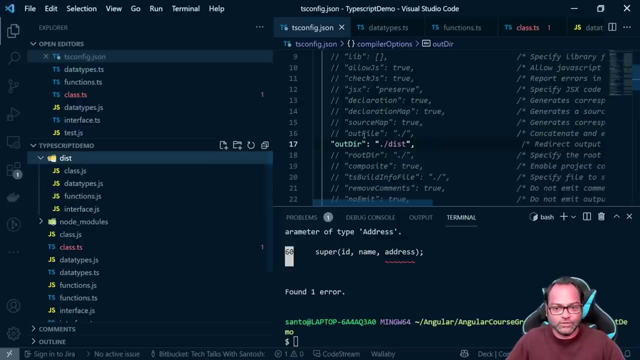 okay, this is the DST folder And now I can just do TSC. And once you do TSC, all the outputs will be generated Inside the DST folder. You can see here all JS files. all the output is part of the DST folder. 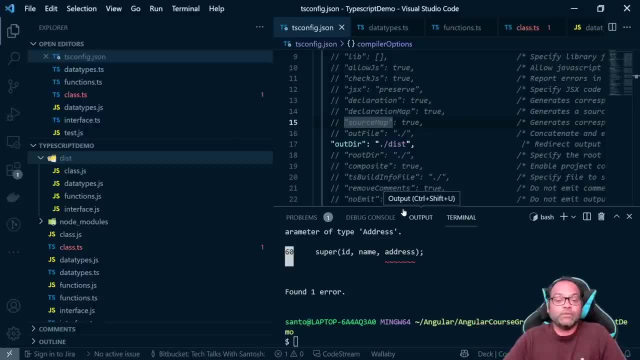 Source map, which is really interesting because, remember I said, we can only run JavaScript on browser. What, in case you want to debug your code? What code we are going to write? Of course, TypeScript. What code we are going to get on browser. 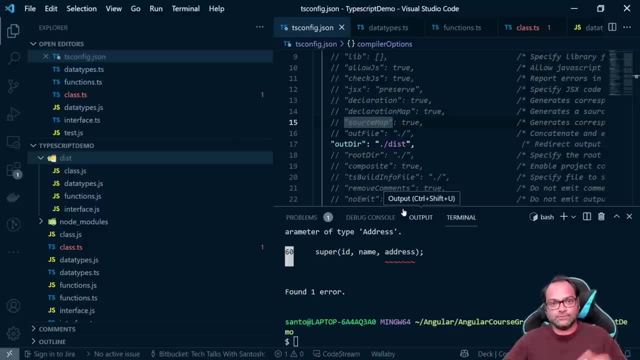 JavaScript. How to debug it? Not possible, right? So, yes, this is possible By enabling the source map. This is also something which you don't have to, because in Angular, in development mode, you will find this property to be true. 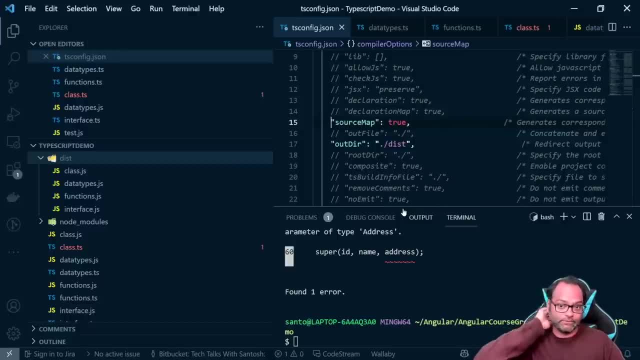 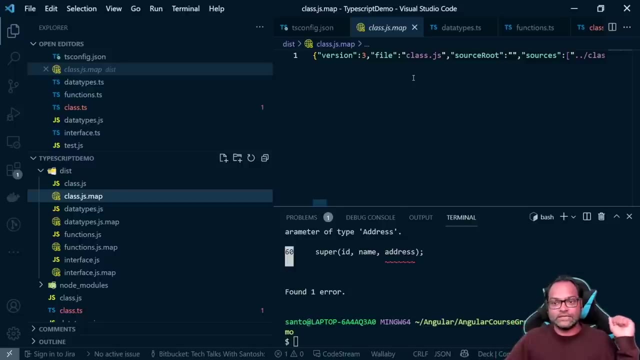 But let's see what happens when you do source map true. So let's run the AC file again. So once we say source map true, a new file, another file will be generated, called map file. This map file contains the information that from where this code is getting generated, 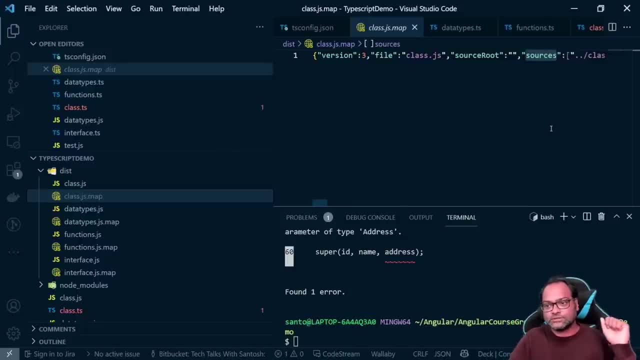 So you can see there is a property called sources, So it's sources. it says it is coming from classts, right? So at runtime, this file will be actually used by your browser to redirect you to the correct TS file rather than JS file. 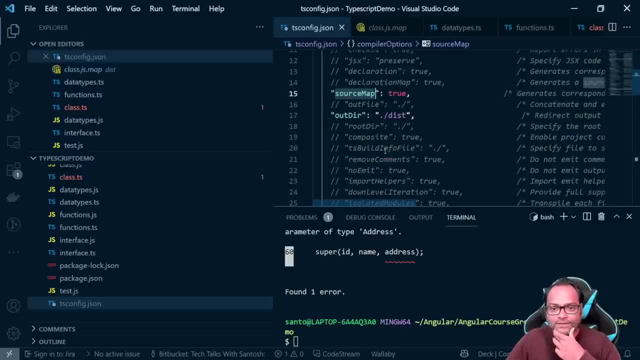 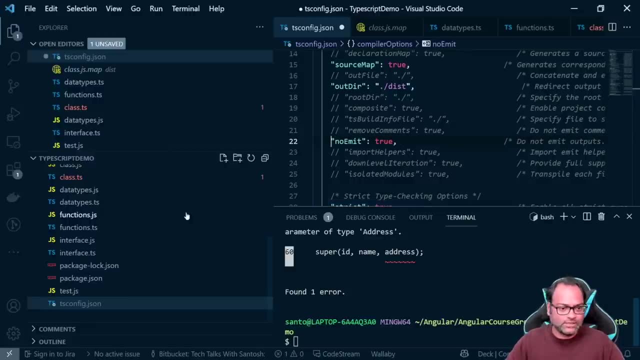 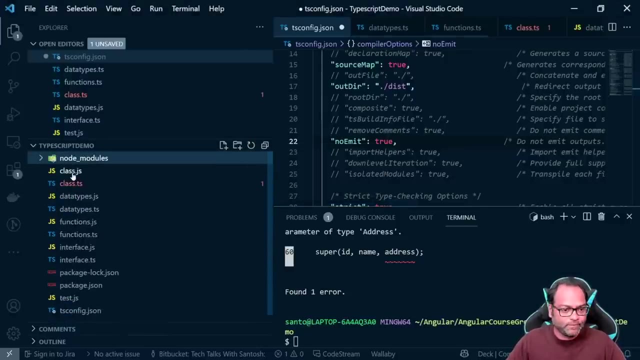 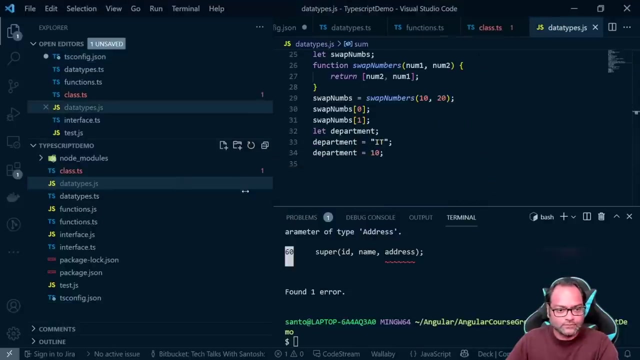 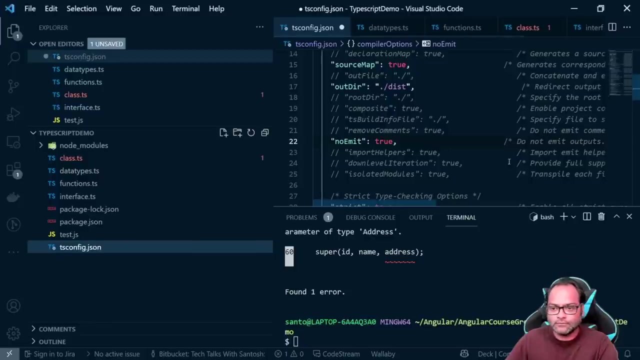 So this is source map And I don't think so you need to know more about. yeah, this is really interesting. I just I'll just remove all the DSD folder, all the JS files. So let's see once you do no emit. 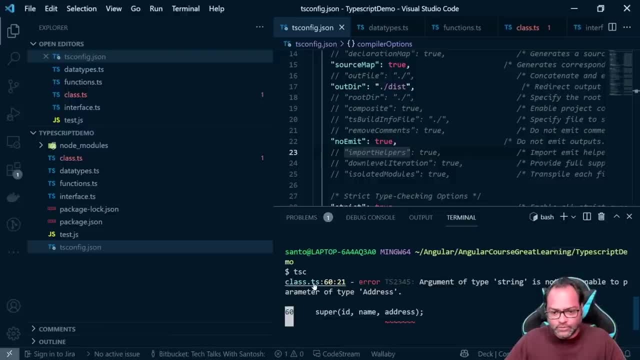 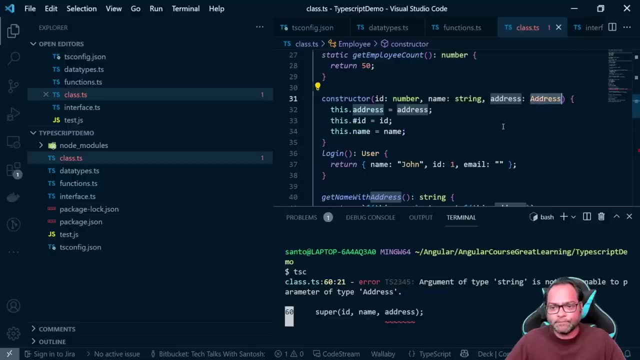 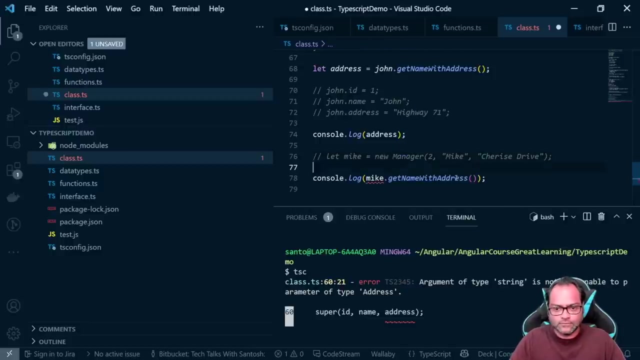 You can see there is no output generated. Let's go back and fix this. I'll just say this is type of address to fix this issue And then we will say this address I think we can get. Let's comment this out of now. 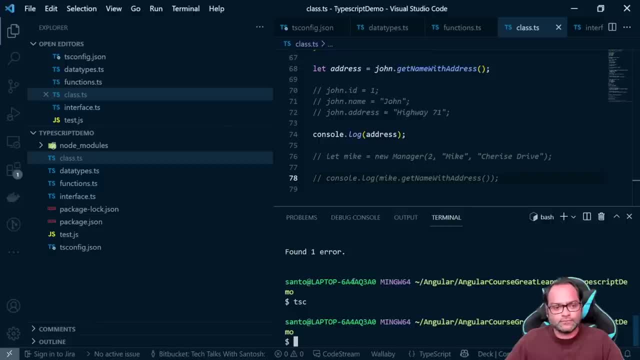 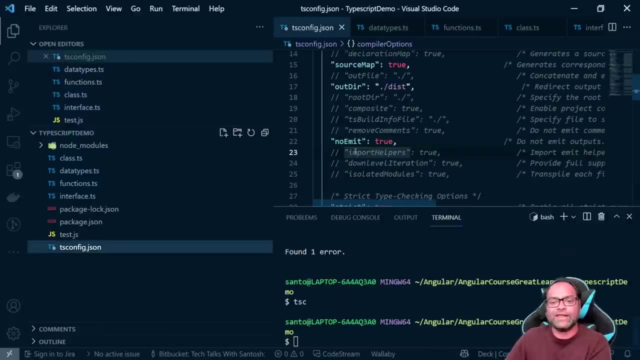 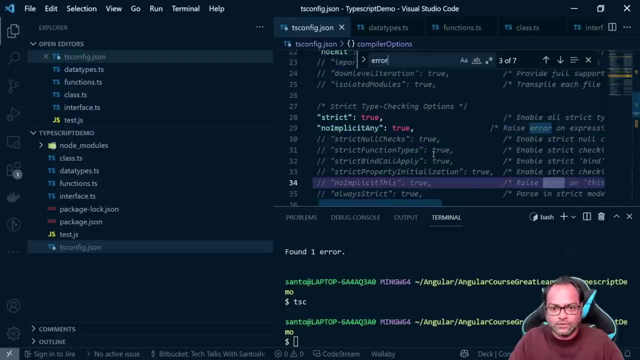 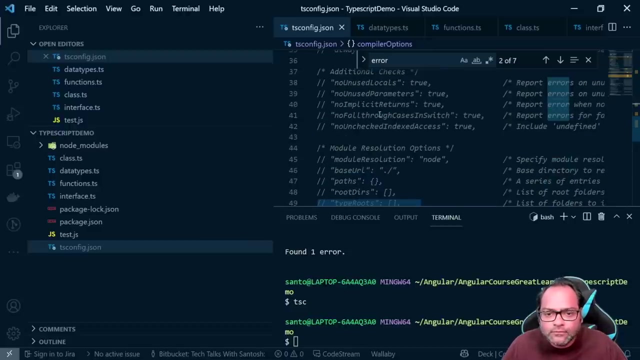 Let's run the AC again. So if you say no emit, then there won't be any output which will be generated. There is another flag. Let's see, Let's look through Sources. So let's move it back to false and let's say TSC. 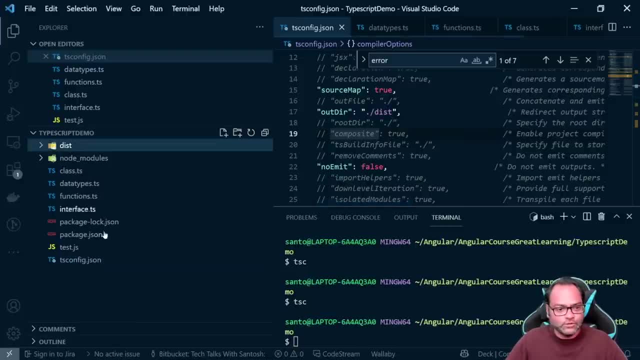 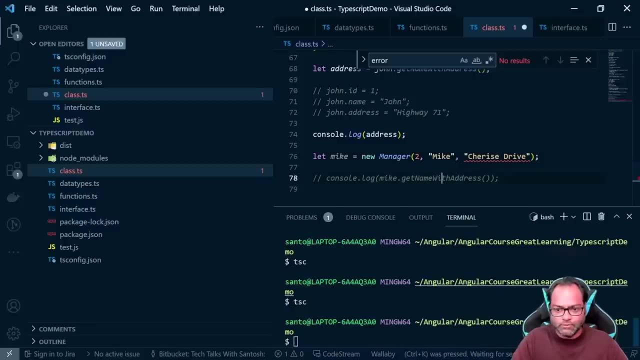 Now you have your output generated. One more thing which I wanted to show you is: let's go back to interface classts. Here we were getting errors right. So, if you remember, if you see this, we are getting an error And once we run TSC, 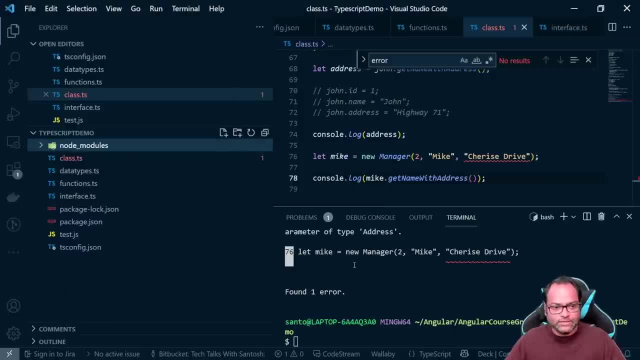 we are getting the error, but it still generates the output. Let's see, I mean, earlier it was already there, So we are not sure if it is generated or not. So let's see, I mean, you can see, even though we are getting the error, 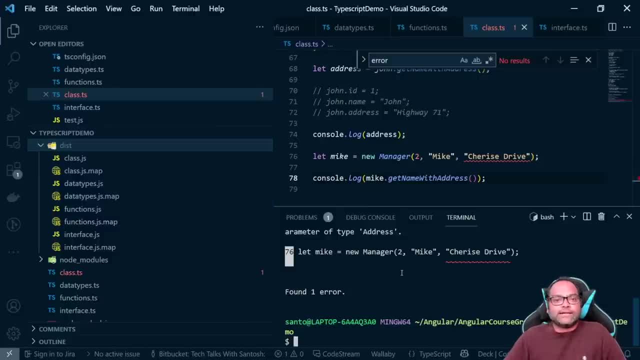 we are still getting the output. So remember one thing: TypeScript cannot stop you from compiling your file. It can only give you errors warnings. Those are like really your warnings. It is saying that, okay, you have some type issue, but it will not stop your code from compiling. 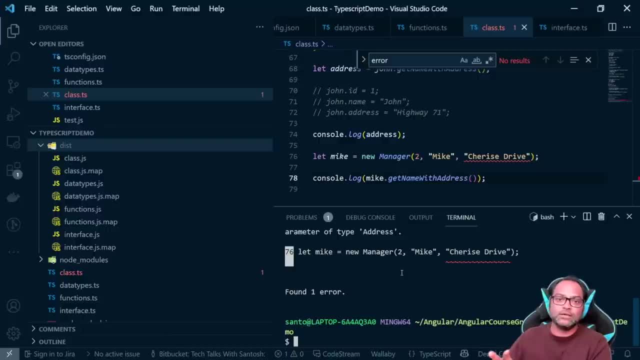 Keep this in mind. So, in case you are like you're relying on this error and considering that your code is actually not compiling- it is not true- Your output will be always generated. It will give you some typing issue, in case it has. 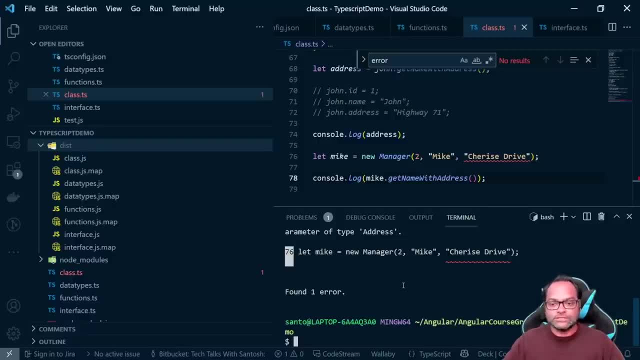 but yeah, it will also give you the output. So this is it from TypeScript section. Now we can go ahead and learn about Angular. All the concept which we have learned is really boring. learned which you have learned. sorry, all the concept which you have learned so far related: 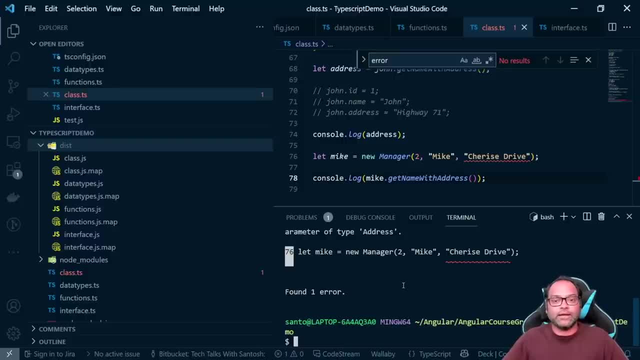 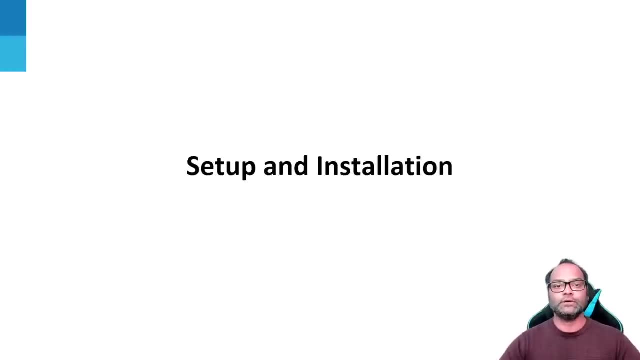 to typescript will be used inside the angular and they are really important, so don't skip anything. so far we have completed with typescript. we learned the basics of typescript. now we are going to apply those concepts, so let's start with angular. so here we will first go through the setup and installation. 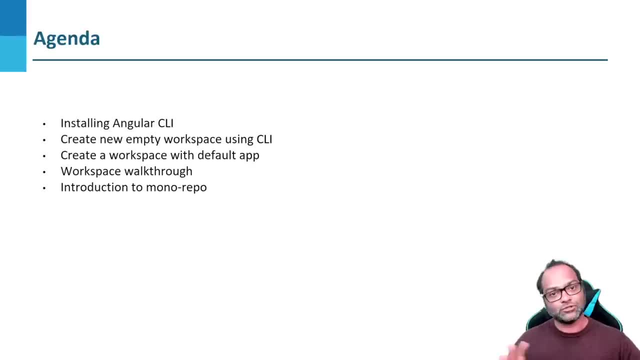 we will set up our workspace and we will install the necessary applications or necessary programs. we will install the necessary softwares required to run our, to run and create our first application. so let's see what we are going to see here in this video. so we'll see how we can install angular. 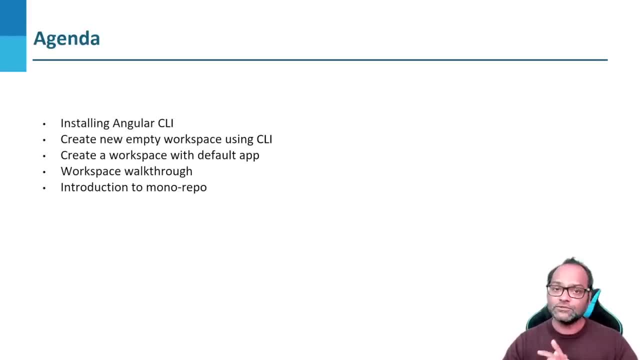 cli. we will see how you can create a workspace using angular cli. we will create a workspace and then we will talk about the files is available in that workspace and finally, we will also talk about monorepo, which is really important. so let's go ahead and get started. in previous video we mentioned that we won't be probably. 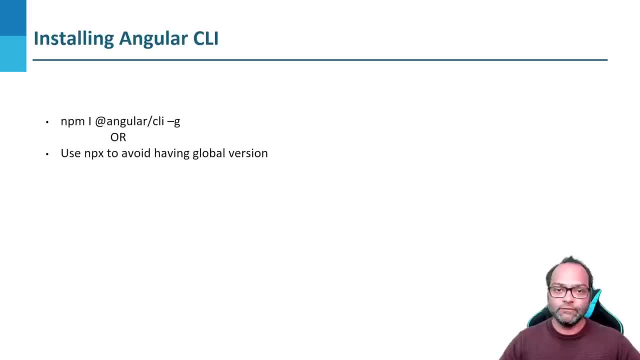 using angular 12, but i think, uh, sorry, in previous video we mentioned that we probably won't be using angular 13, but, uh, we will use angular 13.. i have seen there are not many breaking changes, so let's go ahead and use angular 13, which is the latest version and which will be uh. 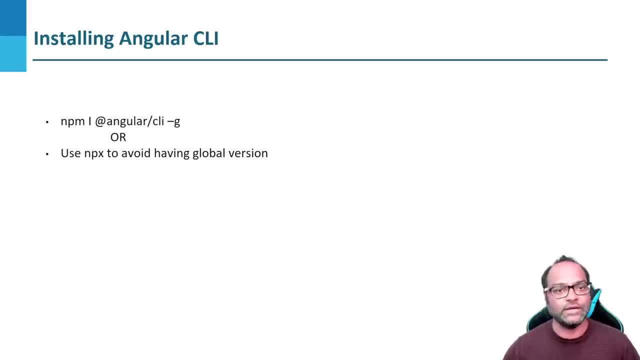 version for next six months, so you will use the same version and it will be easy to even migrate in future. so first thing which we have to do is, of course, go ahead. and, uh, the first thing which we have to do is go ahead and install angular cli, which will help us to create the application. so, 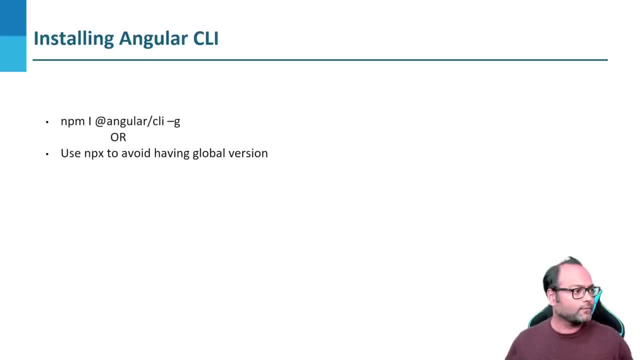 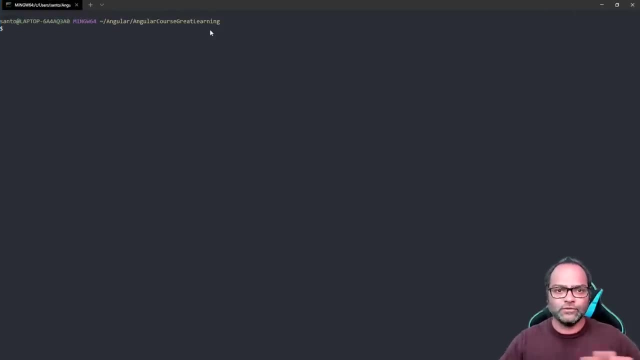 we'll open the command prompt. so this is the folder where actually i'm keeping all the files related to this course. but you don't have to worry about it. you can just open a command prompt and run this command: npm install android angular slash cli hyphen g. so hyphen g is for global, so we 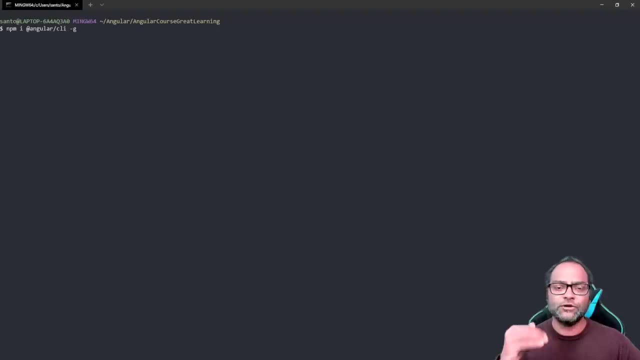 will be installing the latest version of angular cli globally in our machine so you can use the angular cli from anywhere. so you can use angular cli from anywhere on your machine, so you can also verify if which version is installed. let's right now, let's install it and then we'll see how you can verify the version. 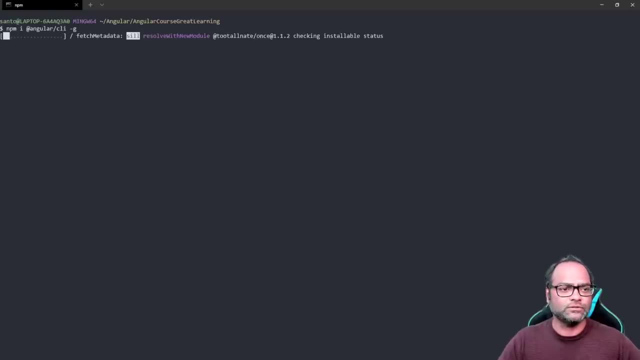 it will take few seconds based on your internet speed. so so it's installed. now you can see. this is the very. this is the version. so it says the angular version 13.0.1 is installed as of now. to see which version is already available on your machine, you can run ng hyphen version which will give: you this version, angular cli version, and it will also give you node version as set. 14 is absolutely fine. angular 13 supports node 16 as well, so in case you have installed node 16, no issue, you can just go ahead and use it. done so once angular cli is installed. 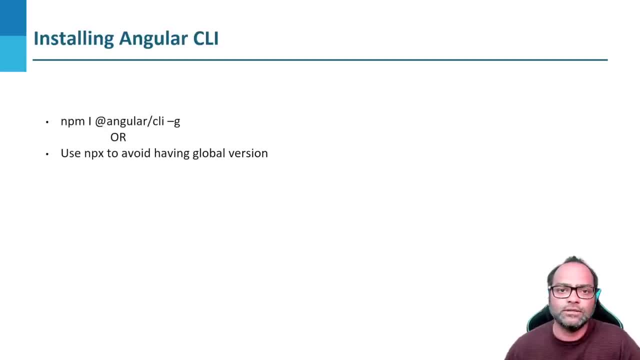 now we can go ahead and create our application. in case you don't want to install the global version, you can also use npx. i'll show you how you can do that. but let's go ahead and now talk about creating our workspace. angular cli allows you to create an empty workspace where you can add: 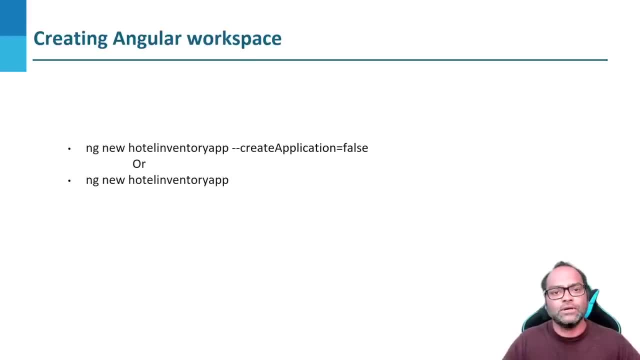 multiple projects and libraries. sorry, angular cli allows you to create multiple projects within your workspace, so you can create an empty workspace and then add projects later, or you can create an workspace with a default application. that's choice is yours. what we are going to do is we will be creating an application with a default application, which we need. 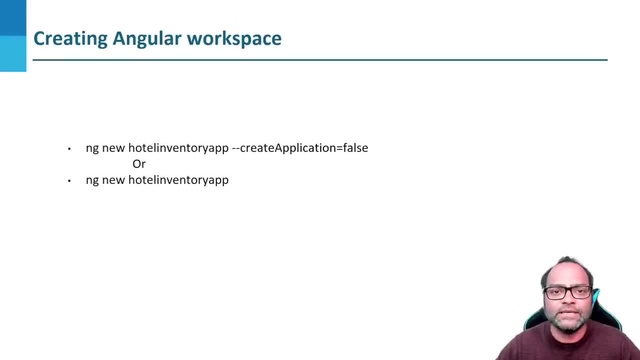 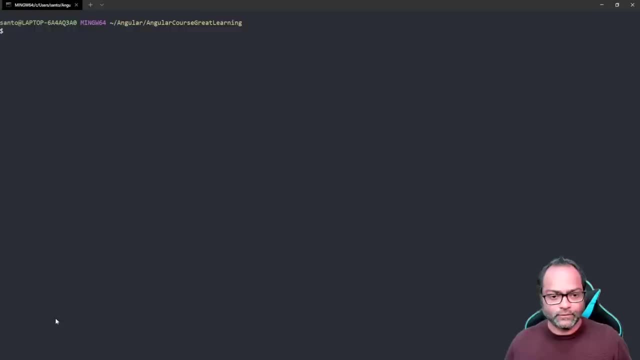 so let's see how we can do that. i mean, how you can create an workspace empty, sorry, how you can create an empty workspace and how you can create a workspace with default application. this is the, so move to any folder where you want to create your project. 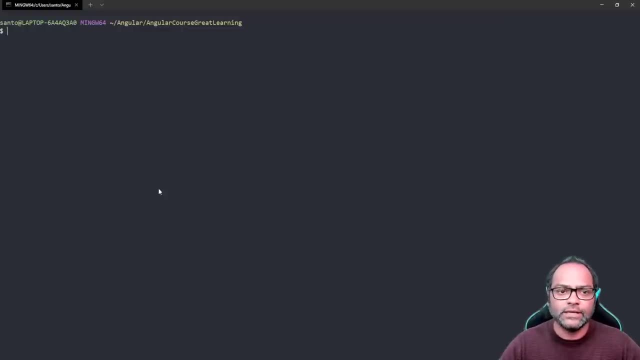 right now i use. i have created a folder called angular and i create all the angular related projects in this particular folder, angular folder. but choose as per your convenience, so you can use ng new command to create a new application. also you can create a new workspace, so ng new, and then you can give your workspace name. i can say hotel. 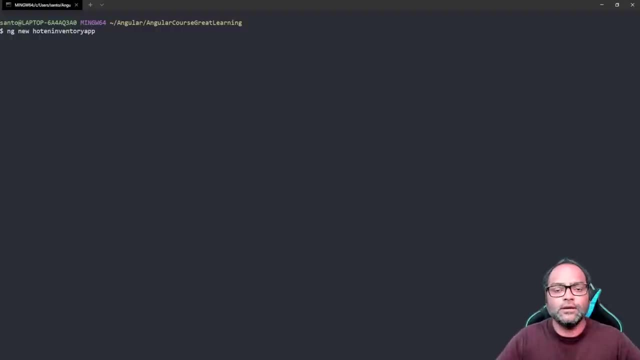 hotel inventory app. as we said, i can create an empty workspace. in case you want to create an empty workspace, you can pass a flag called create. application is equals to false. i want to create an workspace with default project, so i won't be. let's do that, so i'll say: 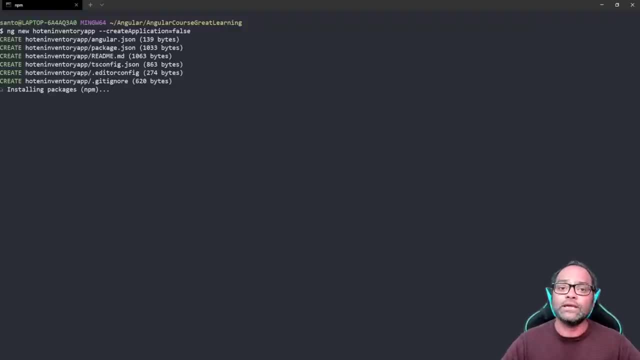 ng new hotel inventory app and hyphen create application equals to false. this will create an empty workspace for us, so we will delete it and then we will create again with default project. so right now it is installing the packages. i'll just cancel it here because i don't. 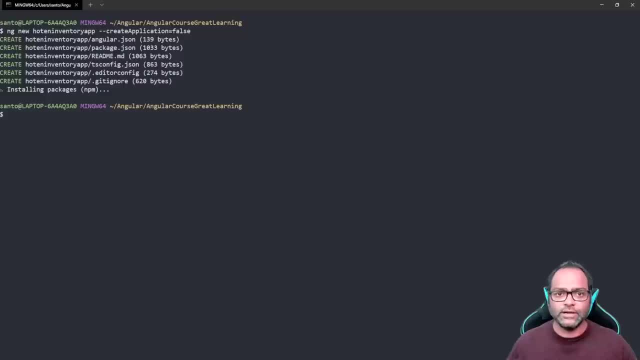 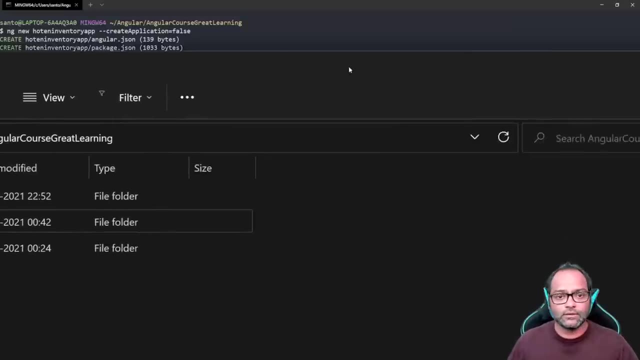 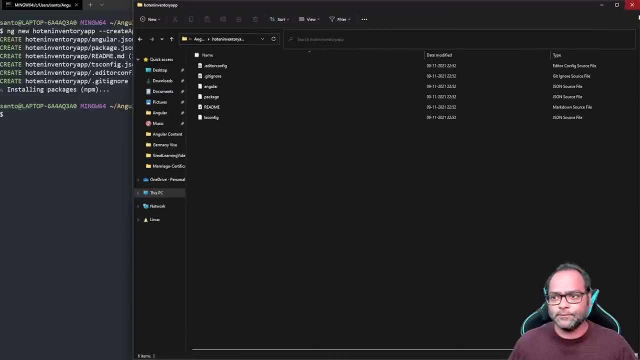 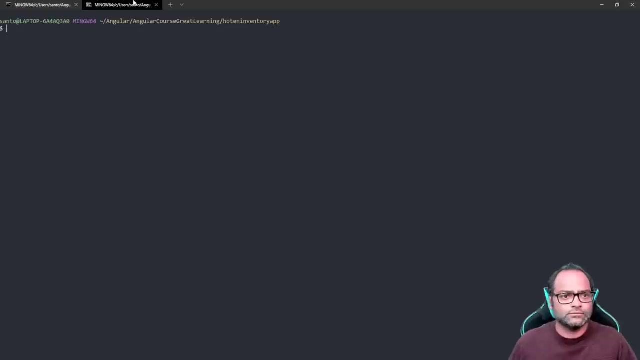 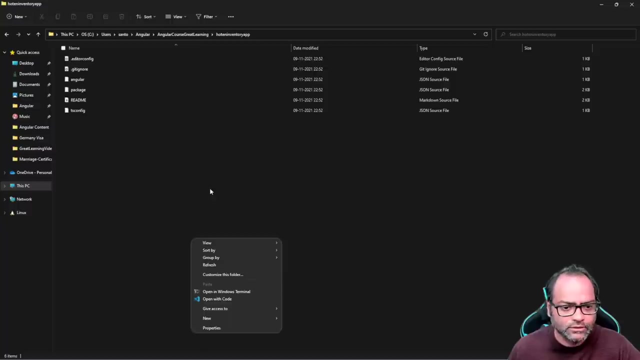 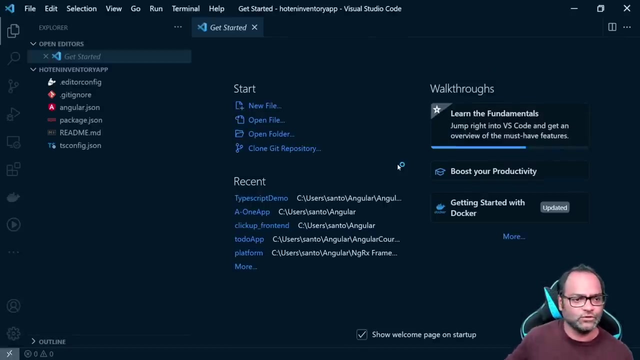 want the packages to be installed. i can, because i want to delete this folder and then create a new. yeah, so we want to create a new application with with a default project. so here we'll just open this and open with code, so we'll see what we get when we create an empty workspace. so you can see, i we don't have uh much uh files. 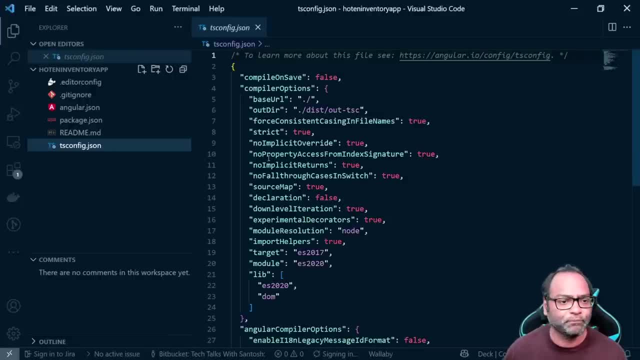 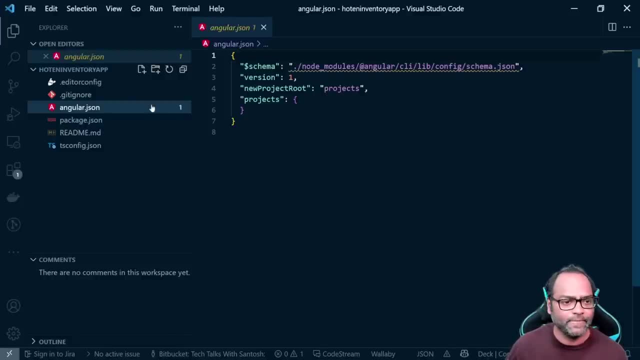 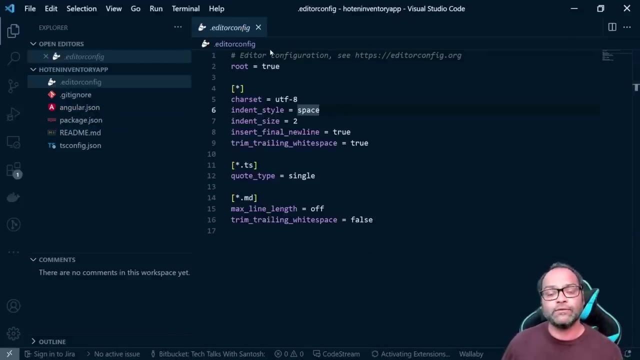 available here. you have dsconfigjson, which we have seen. we have packagejson, which we have also seen, angularjson, which is like angular json, angular's configuration file, and uh. rest of them are just readme and gitignore and editor config files. so this is it. this is what you get once you. 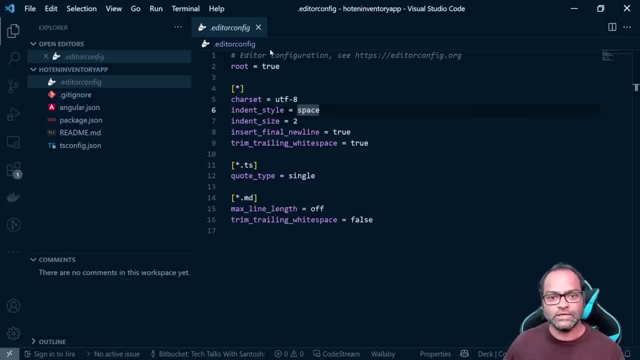 create a workspace without a default application. now you can add a application as well. let me show you how. and that will require us to install the packages. so let's go ahead and do that, and just don't need to do it, but let's see. so to install the packages, you can run nbmi and it will read all. 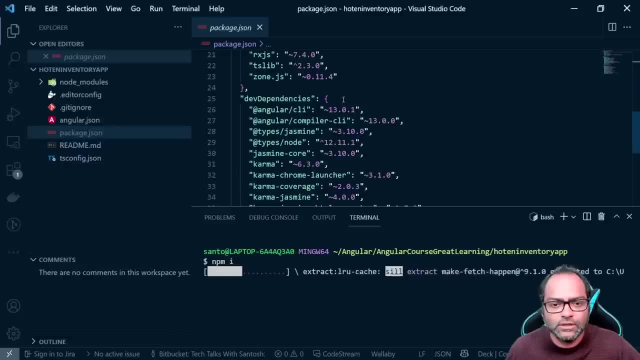 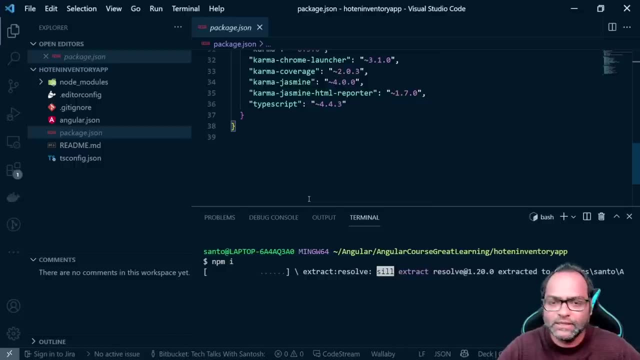 the packages which is required from packagejson and it will install, and then we'll see how you can add a project into this empty workspace and then we'll delete it and then we'll create a new workspace with a default project. okay, so now it is installed, so let's see how to create a new. 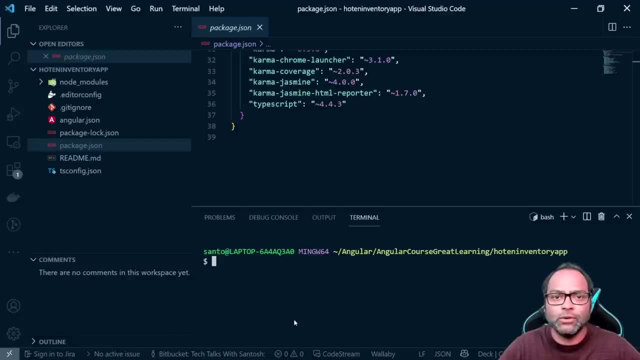 so what we want to do right now is we want to create a new application so you can use ng generate app, which is short for application, and your application name, which is, let's say, hotel. so this is our application name. a hotel inventory app is our workspace name and it will ask if you want. 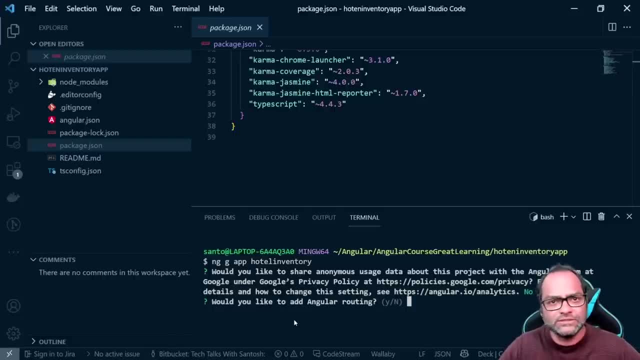 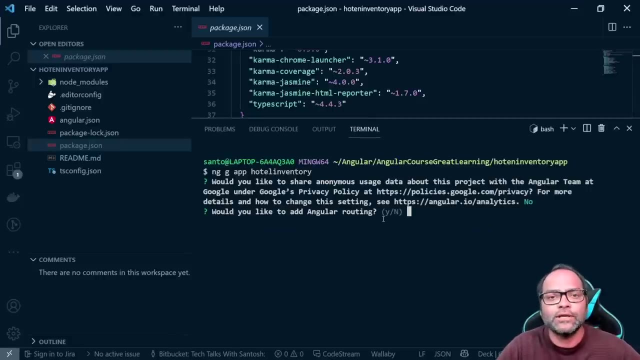 to actually share this information with. i mean, this is just for, like, usage of the commands, so it's up to you. so this will ask some question whenever you create an app. let's see those questions. so it says: would you like to add angular routing, as we are going to? 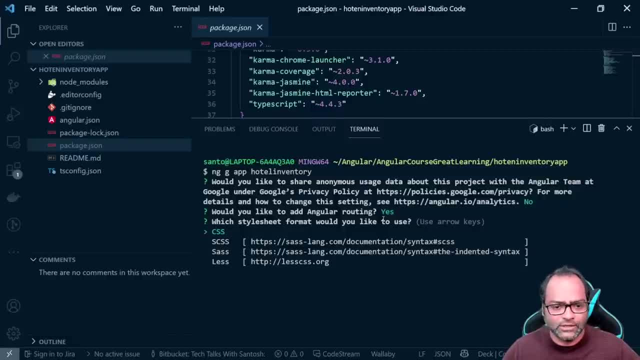 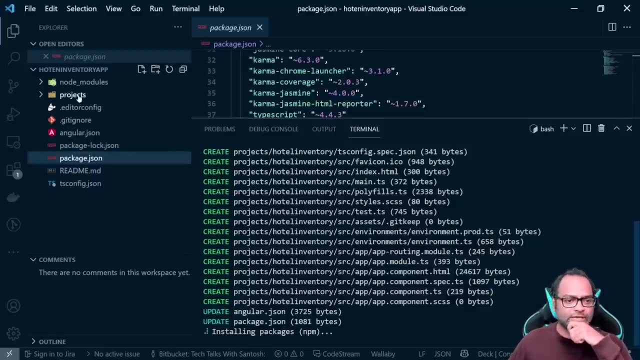 use angular routing. later on i'll say yes, don't worry about it right now. uh, which stylesheet you want to use, i will go with the sas, and this is it. so you can see, a new project has been created here called hotel inventory, and it has some files. these are the files which we'll talk about. 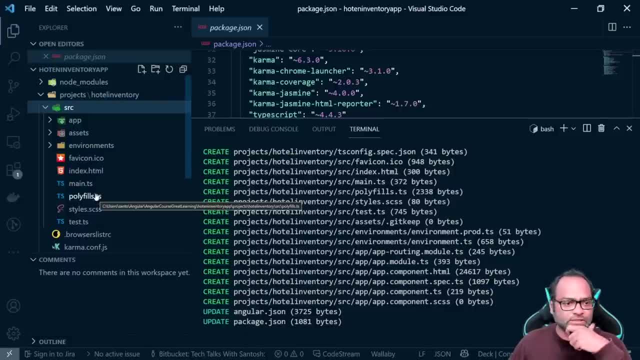 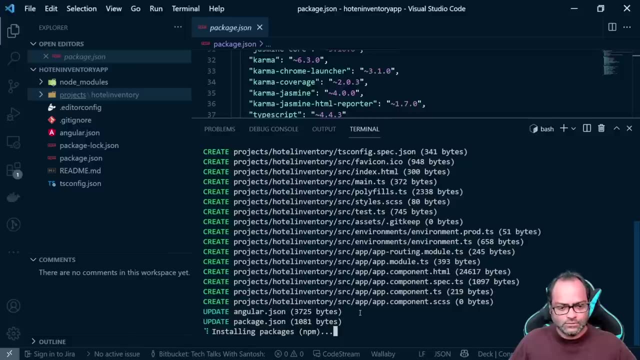 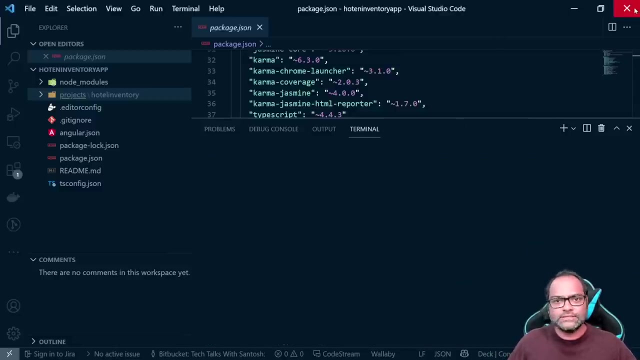 later on, later, once we finalize our workspace. and now we can just skip this installing packages thing. yeah, so this is how you can create an empty workspace and add project later on, in case you want to. and now let's see the other way, where we will create. 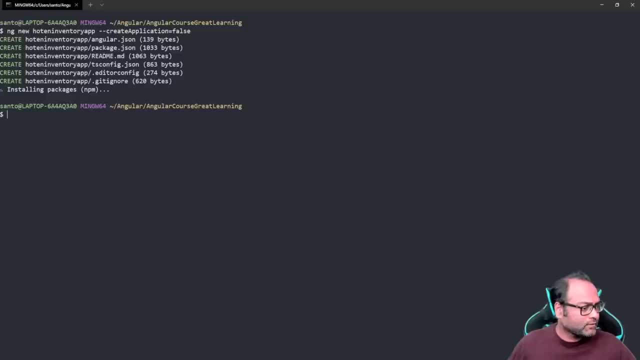 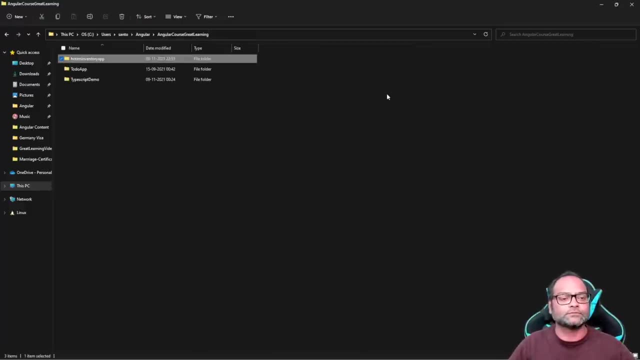 a workspace with a default project. so first i will go ahead and delete this folder and then paste it in the folder where we are going to say that this is our workspace. okay, so i go back in to my database and i will just go ahead and add a new project. 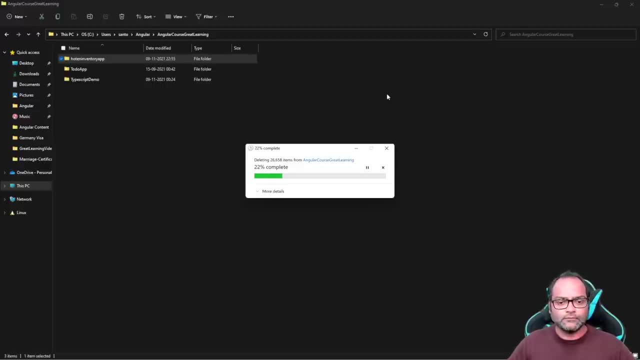 and i'm going to go ahead and click on my SeiCi 365 file and a bunch of files, but i'm going to go ahead and copy that into my new playlist and i'm going to this playlist and i'm going to go ahead and do a quick research and there we go. okay, let's go ahead and I'll. 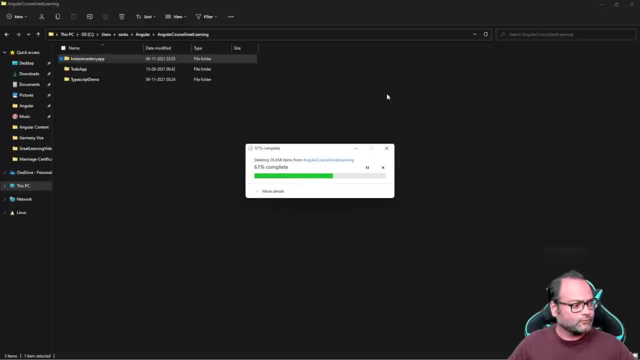 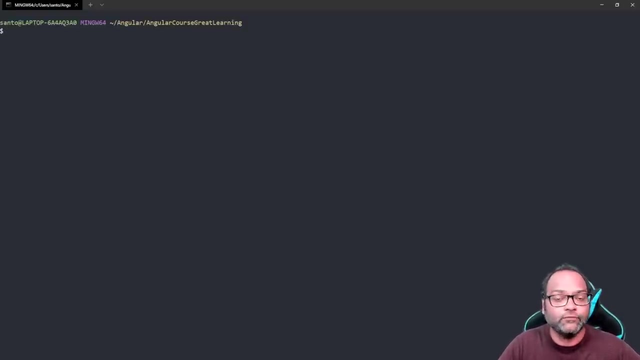 just put this on the website so i can go here and i'm going to go ahead and click on a project. So now, once that folder is created, now let's create a new workspace with a default application. as I said, We can say ng new and you have to just mention the project name So I can say hotel. 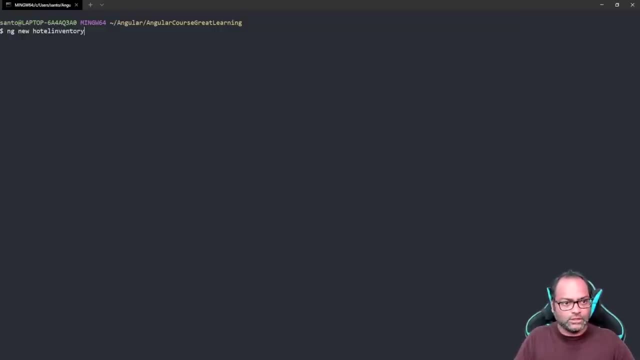 app and that's it. You don't have to mention hyphen fn. create application flag and this will create it. will ask you the same question: whether you want to add routing. We want to actually use routing in future, So we'll say yes. Which style should we want to use? I'll say CSS and that's it. 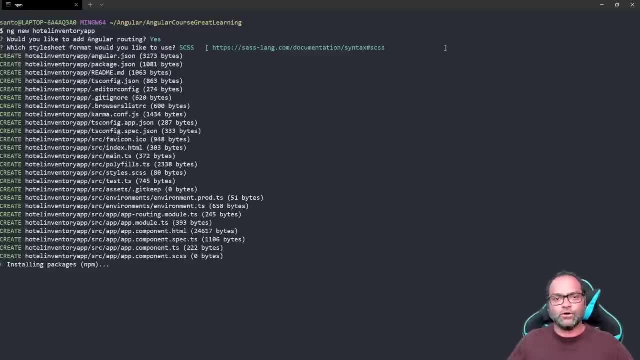 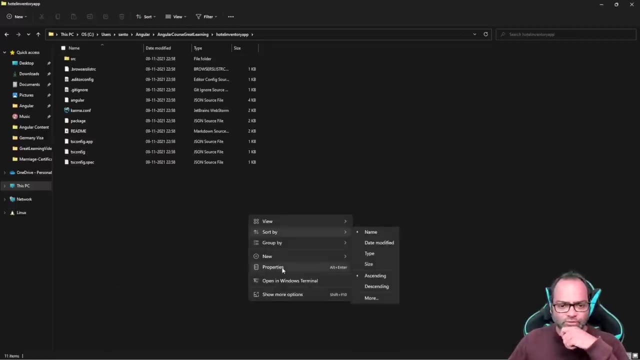 Now it will create your workspace with default application or default project. So now all the files are already generated, So you can see hotel inventory app, and now only the installation is going on. So meanwhile, let's go ahead and open this project in our VS code. 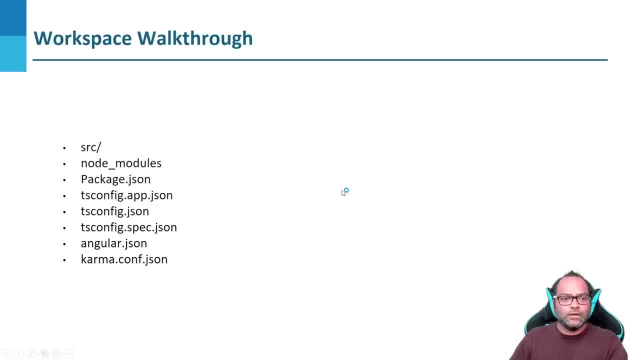 Okay. So now the first step is completed. We have learned how to install Angular CLI and how to create an application with default project. without default project, I mean an empty workspace where you don't have any project, or a workspace where you have a default project. 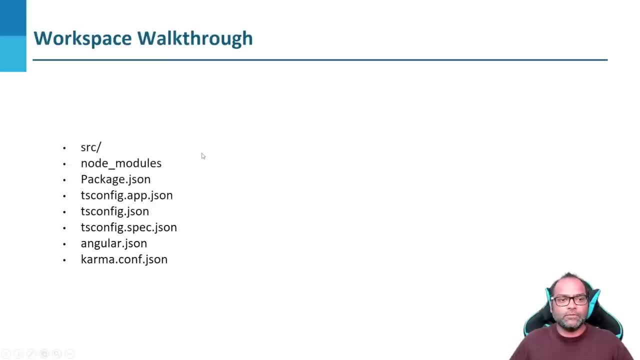 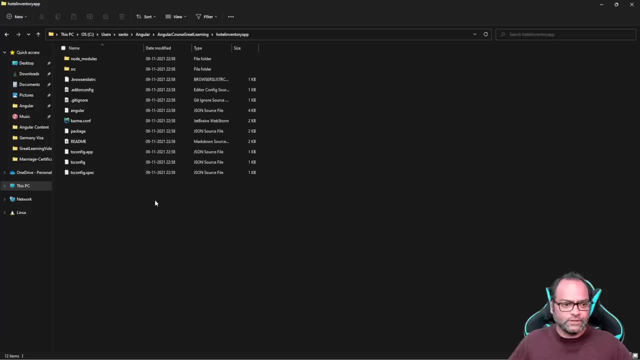 So now, next, what we need to do is we will learn about what are the files which is available within the workspace we just created. so we'll start with the last one. we'll start at the bottom and then we'll go up. so let's see what are the files which is available. 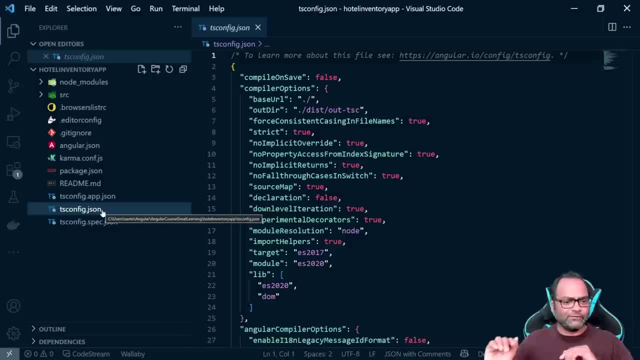 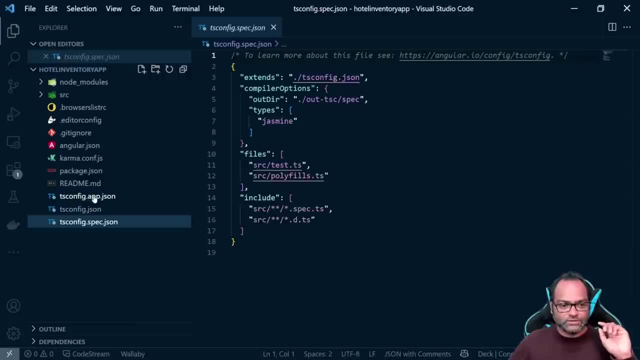 so the first file which is available is tsconfigjson. you might be wondering why i'm not saying tsconfigspecjson, because that's the first file which is here, right? so there's two files: tsconfigspec and tsconfigapp. they both extend tsconfigjson. you can actually verify here. 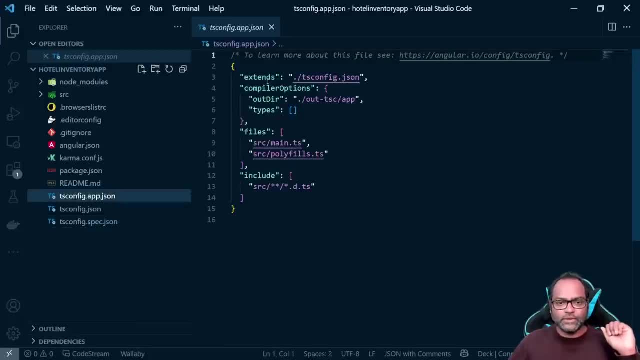 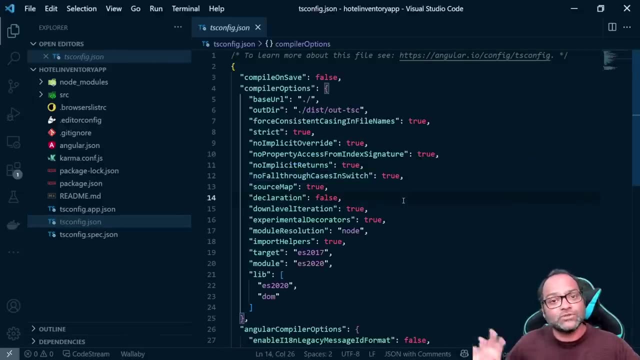 the first line extends, and even if i just open app, it will also say extends. so what is the purpose of these two files? so let's first talk about tsconfigjson. so this is your ts configuration file, which we learned during typescript. you may see there are few. 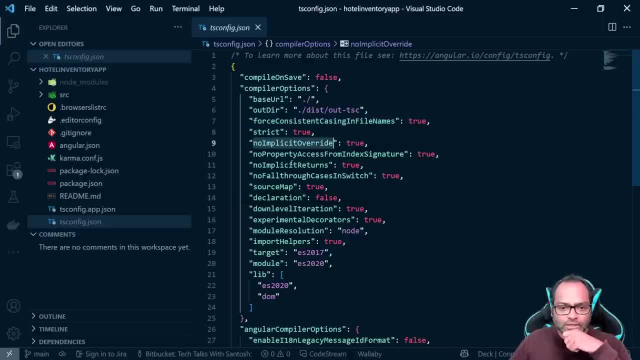 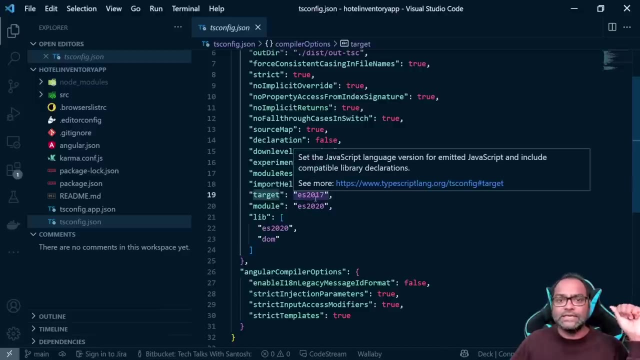 things like strict, no implicit returns. so these are all flags which is available in typescript and source map. then we had target, remember? so now we said we we were using es2015. now angular is saying es2017 is safe to use. so that's it module. we said es next. 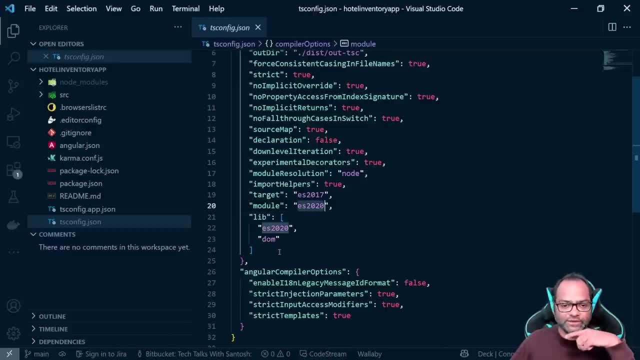 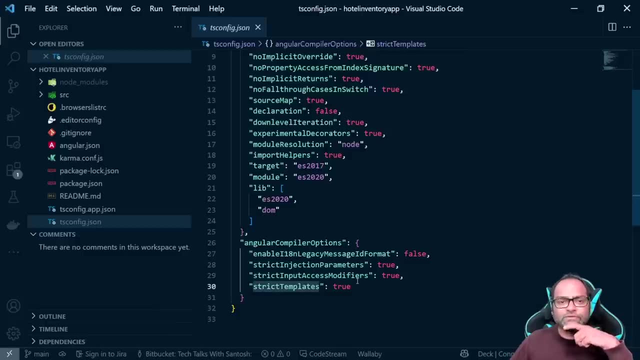 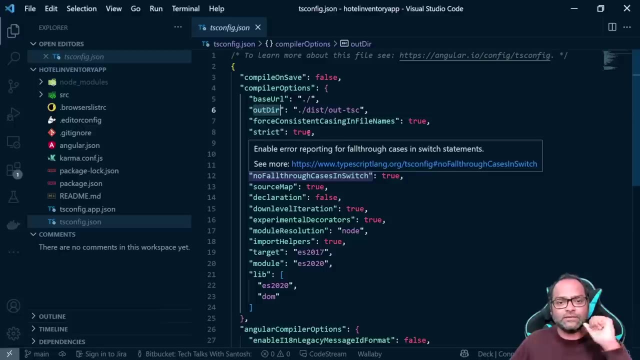 but yeah, here it is to es2020, so which is absolutely fine. and then there are some angular related flags which will, uh, which will be used internally by angular- we don't have to worry about it right now- and then you have out there, as we see, as we have seen right where, all the outputs. 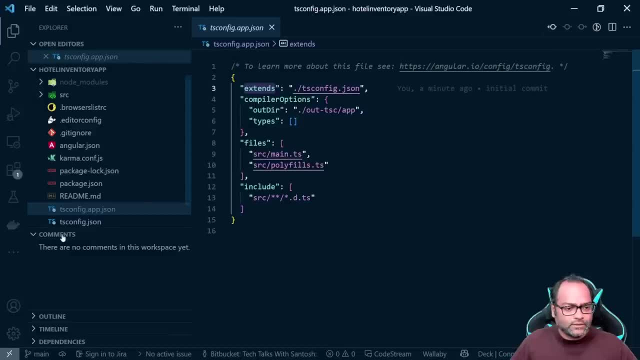 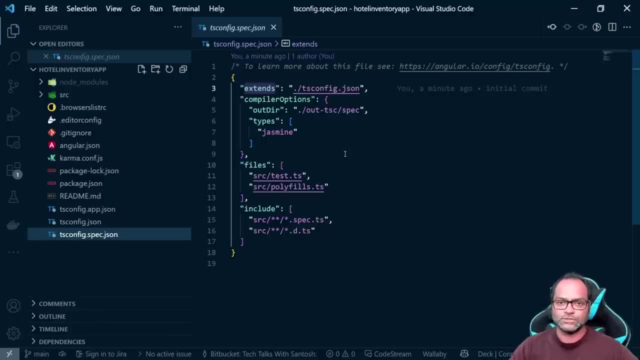 gets generated. and now, whenever you write code in angular, you will be writing two types of code most of the time. so you will be writing application related code and you will be writing unit test. angular says all the unit tests which will be automatically generated for you. we will be seeing some command which will generate all the files. you don't have to. 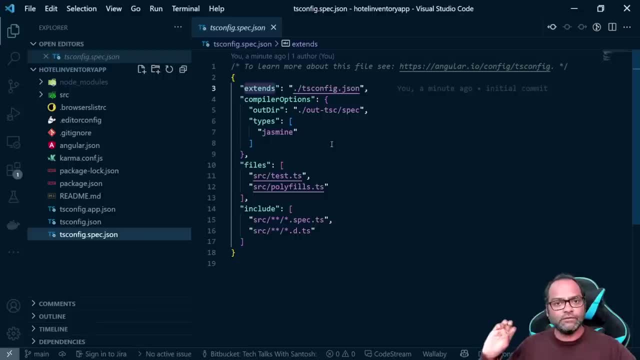 generate files manually, so everything will be generated- will be created using angular cli. subject: » » » » » » » » » ». Our files will be generated by Angular CLF for us And this specjson will be used by all the unit test files. 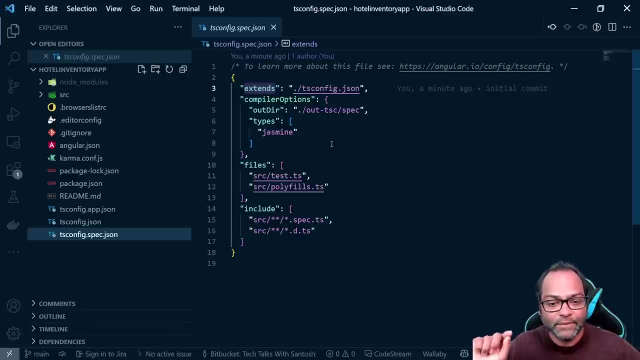 So Angular generates all the unit test files named as specds. So you can see here it says include specds. So all the unit test files will be named as specds And this configuration file, tsconfigspecjson, will be used to compile those specds files. 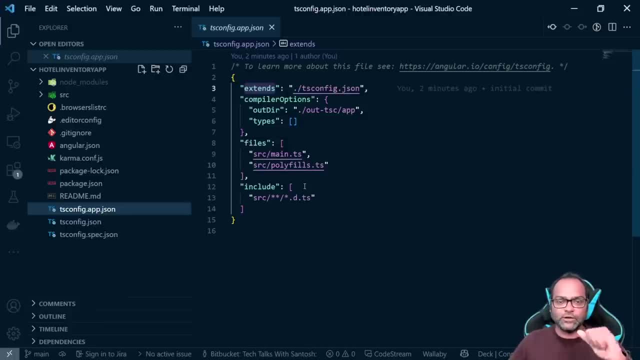 And you will be writing the rest of the code, which is like ds files, which is our application code that will be compiled using tsconfigappjson. So that's the only difference. So now, as we know about tsconfig files, let's move on. 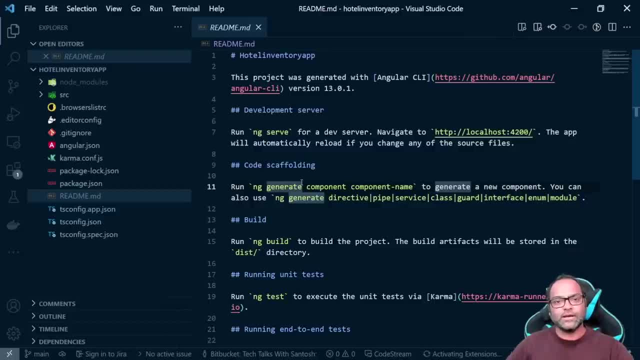 So readmemd is our application code. readmemd is something which will be used only for your repositories. For example, if you upload your project on GitHub, GitHub actually displays all the information from your readme on your repository. Let me show you quickly. 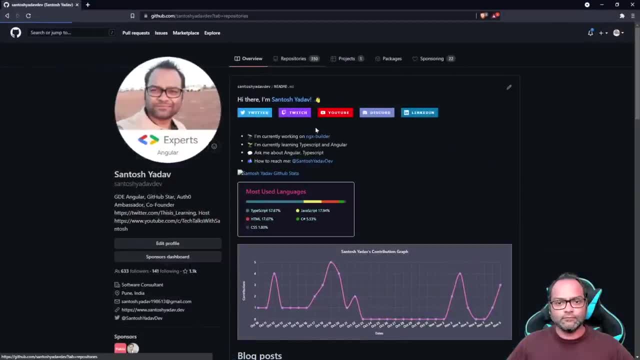 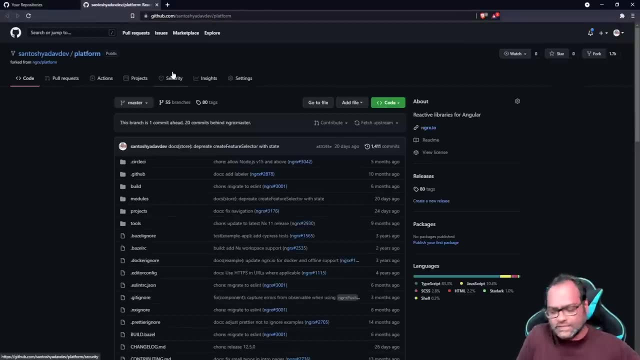 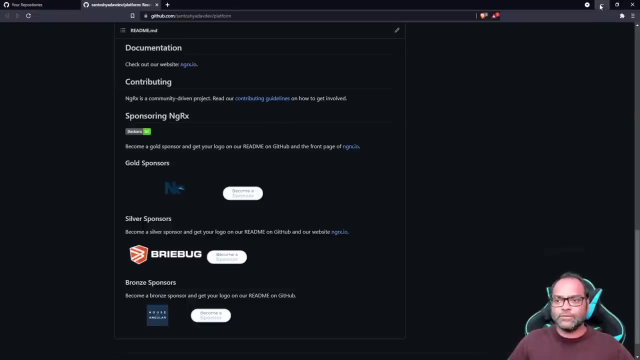 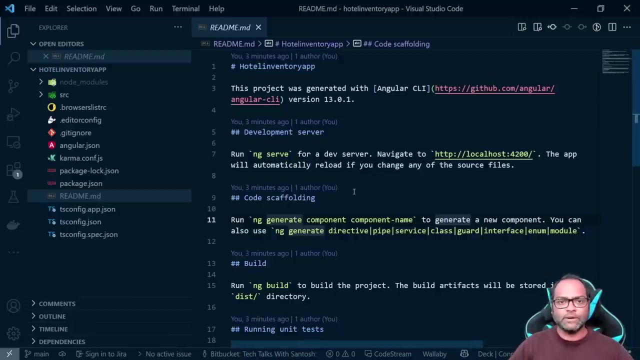 So this is ngRx code base, So you can see here all this information is actually coming from readmemd. That's the purpose of readmemd file, where you can give some information about what your project is. what are some commands? for example, building your application, testing your application. 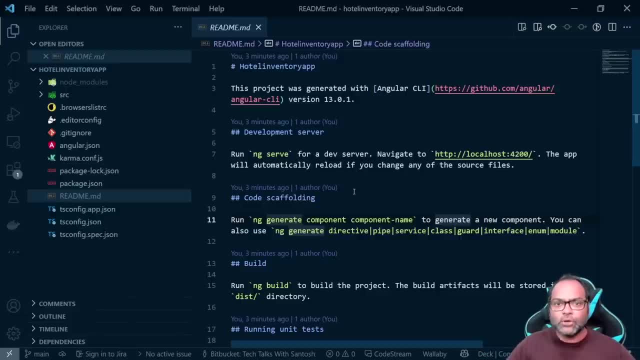 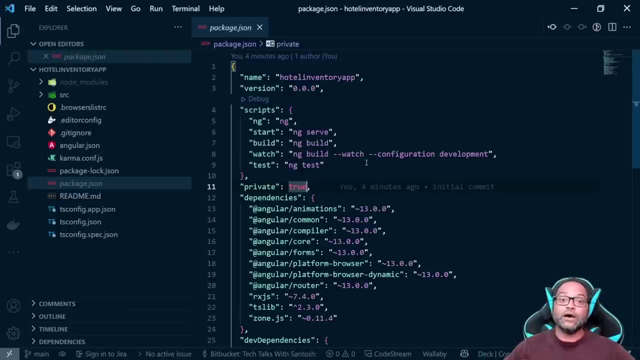 So you can mention all those to make contribution to your project easier. Then you have packagejson. So here we will have all the packages which we are using, And there is two things. I mean dependencies and dev dependencies, which is available here. 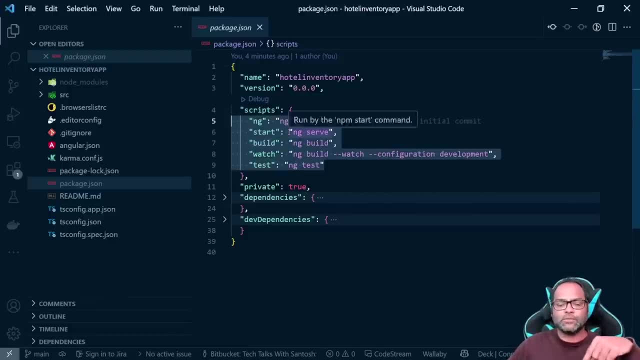 And there are a few commands which will be used, for example, how to run your application locally, how to build it, how to run tests, And you can also run it in watch mode in case you want to. So it's up to you. So a lot of developers get confused between dependencies and dev dependencies. So it's easy to actually identify any packages which will be used And needed for your production build. goes into dependencies Any packages which is just for your development purpose and it won't be part of your production. 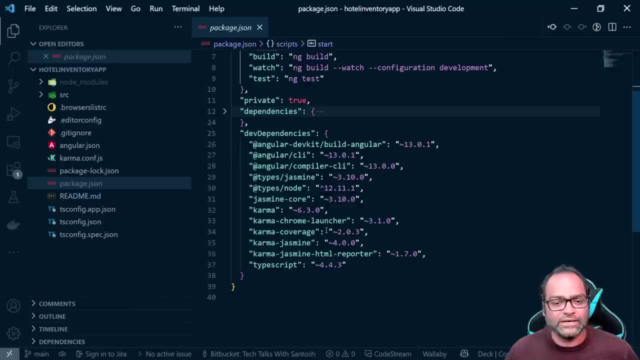 build goes into dev dependencies. So, for example, all the packages related to test, Karma, Chrome Launcher, all these packages are actually your dev dependencies, Even TypeScript. even though we will be writing our code in TypeScript, TypeScript is not your dependency because we are not going to deploy TypeScript on production. 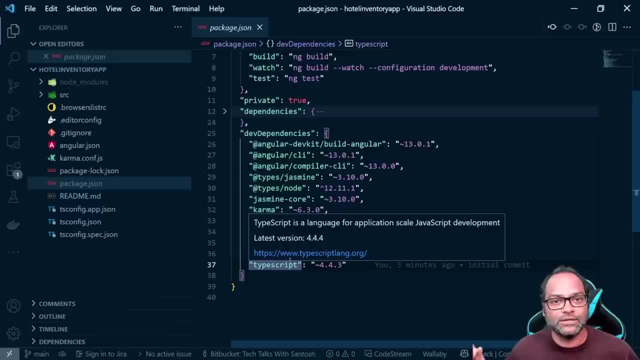 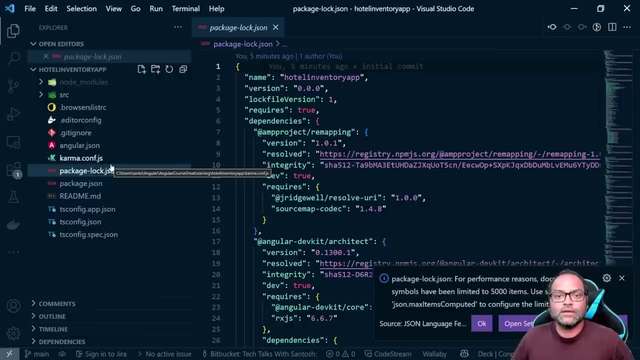 On production. We will be, of course, deploying JavaScript, because the browser only understands JavaScript. Log file is something which is used by CI. in case Log files are generally used by your CI environment, It is optional. It's up to you whether you want to use log file or not. 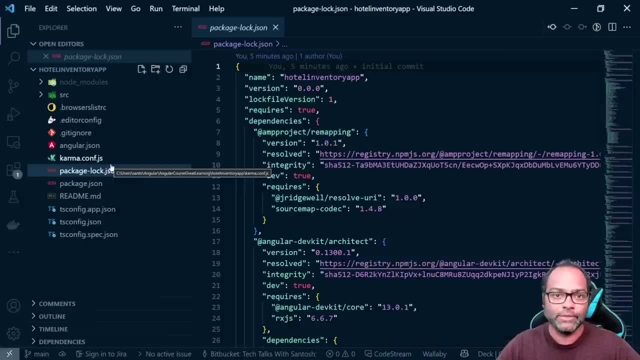 In big teams it's always good practice to use log files, But in case you have a small team, I think prefer deleting files. It's absolutely fine. The problem in large teams is that so many developers will be adding new packages, removing. 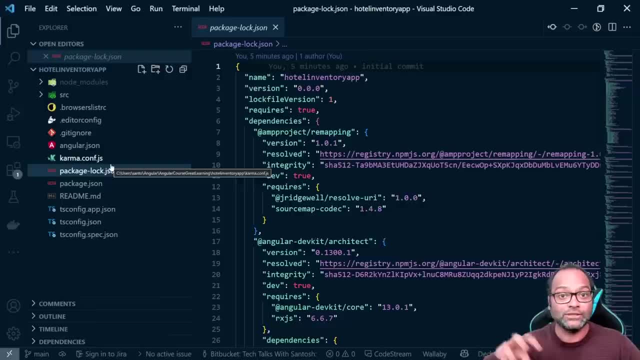 new packages, So log file. make sure that you all are on the same version. In case someone changes the version, they have to commit log file. The only overhead is: in case you add new packages or you update any packages, log file needs. 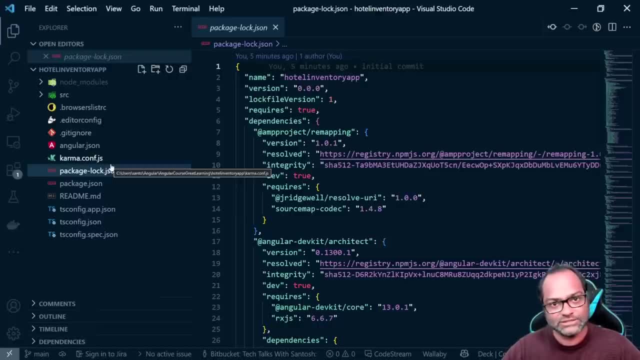 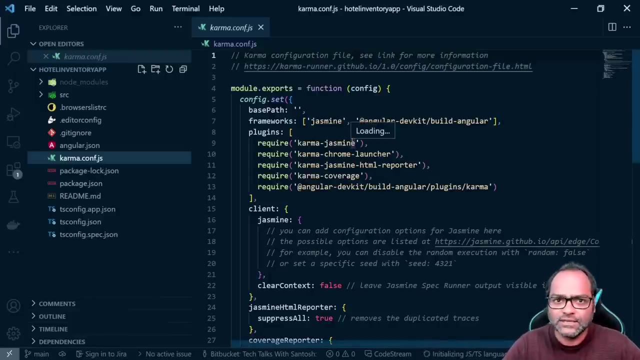 to be updated as well, Otherwise your CI will fail. Then you have karmaconfjs file, Which is anything with configuration, not conference. So karmaconfjs karma is actually a task runner to run your tests, And Angular comes with a default unit testing framework which is Jasmine and Karma. 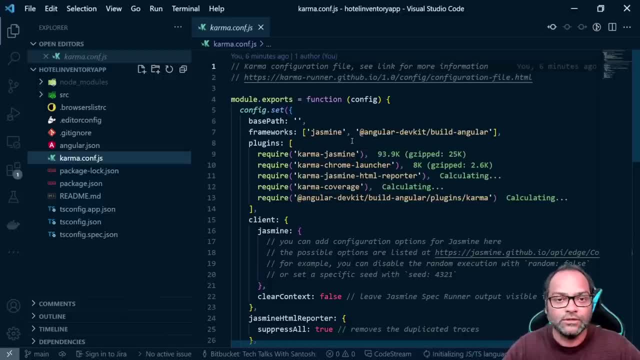 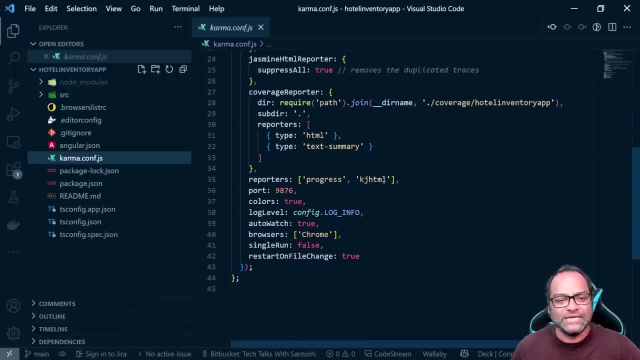 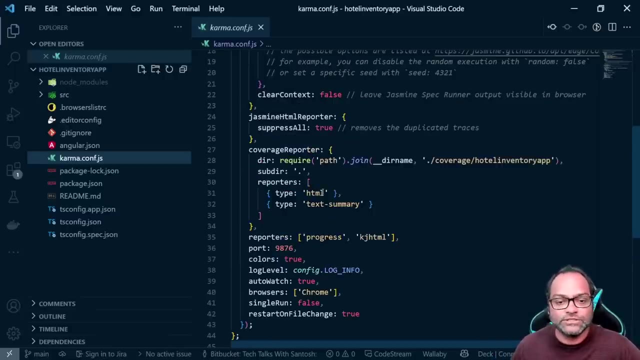 So you'll be writing your all test cases in Jasmine and then you will be using Karma to run those tests. You don't have to change anything here until you need to. for example, you can change your threshold values And you can add more of this coverage or coverage reporters, it's up to you. 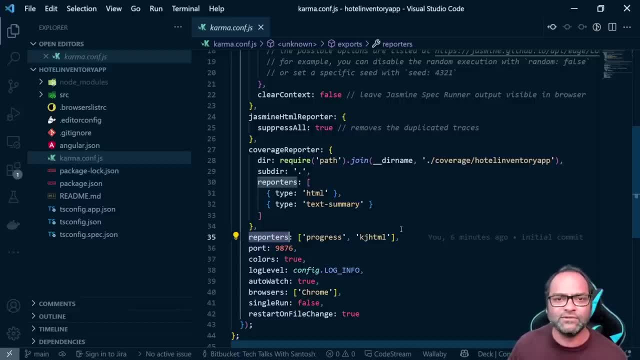 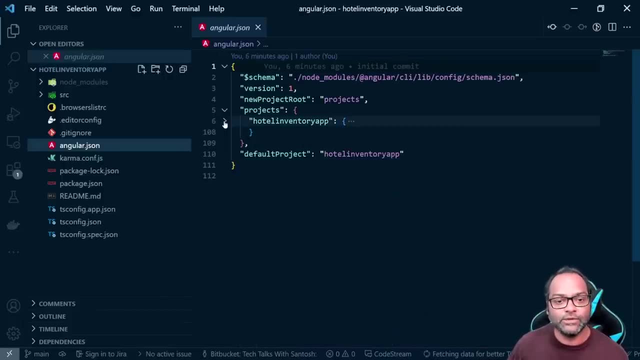 I mean, you can read more about it from Karma website itself. you don't have to go anywhere else. Angularjson will have information related to your workspace. For example, right now in my workspace there is one application which is hotel inventory. 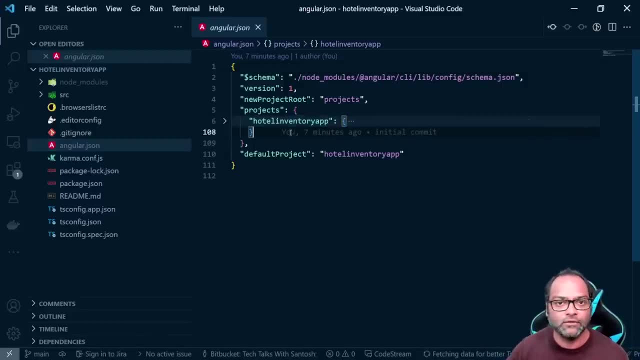 app In case you add more projects. this config, this Angularjson file, will have a lot of information related to your workspace. For example, right now in my workspace, there is one application which is hotel inventory app. So you'll have all this information about every project, each and every project. 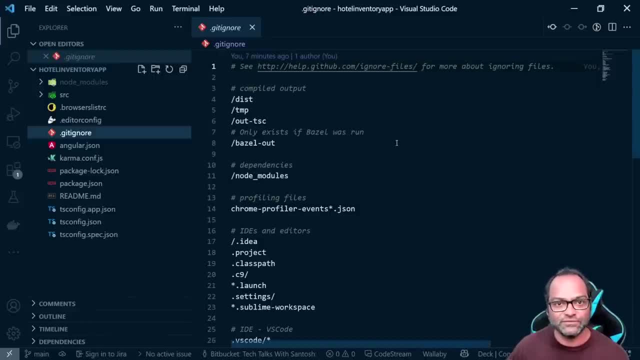 gitignore is a file to ignore some files which should not be checked in, and you can see here we have node underscore modules because this node modules should not be checked in. Never do that. I mean it's like some node module should be installed every time whenever you are. 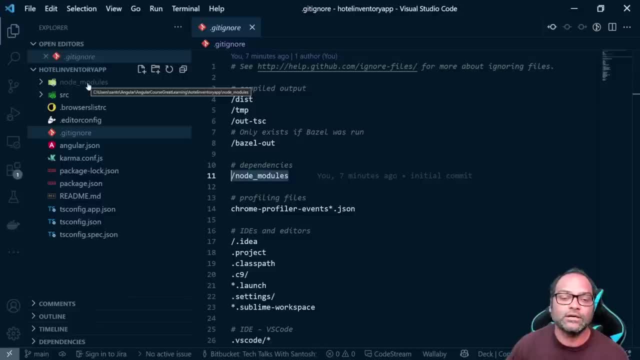 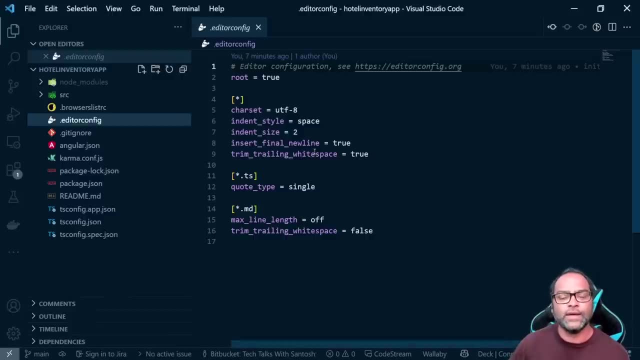 running it on CI or if someone takes the latest project so it should not be checked in. And then you have EditorCopy. Ok, editor config. it's like: uh, you can. the advantage of having enter config file is the advantage of having a config file is you can actually uh, set up your environment, your local editor, based on. 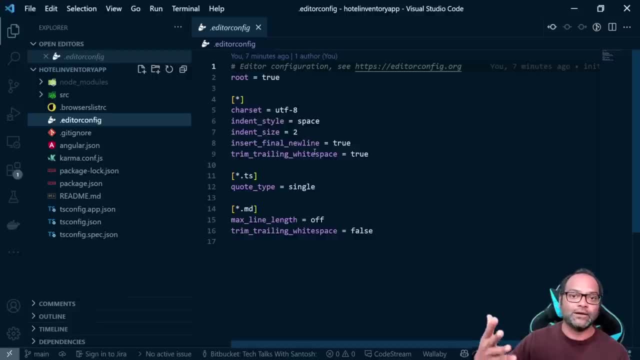 some settings from any other editor. for example, you are a big fan of some other editor- right, atom or webstorm- you can bring some configurations here. so that's the purpose of having editor config, which is it will allow a lot of other things to be generated in your browser list. 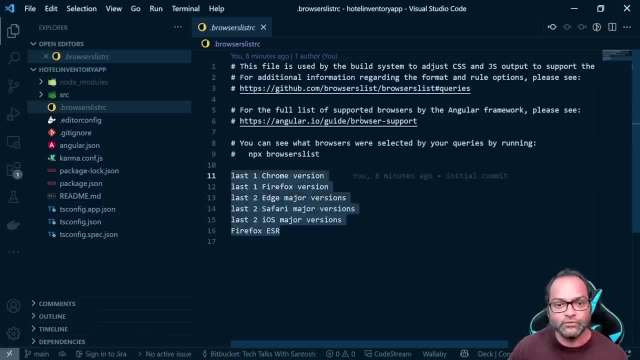 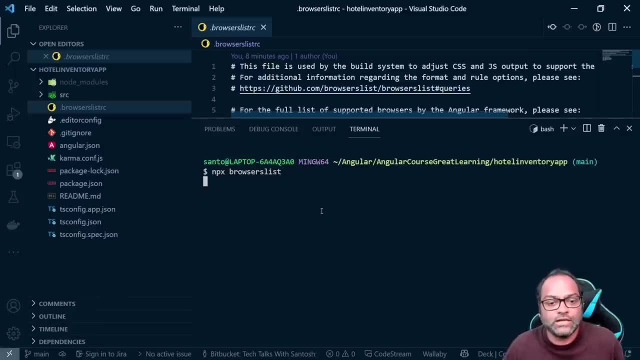 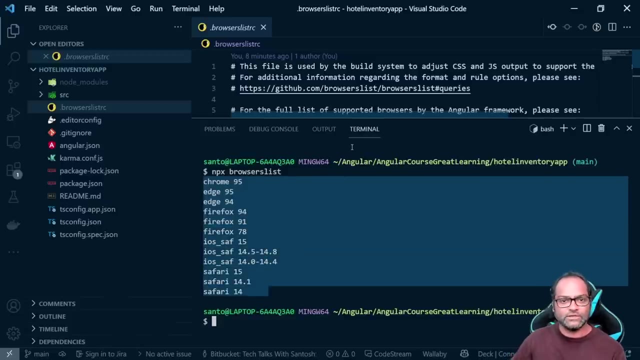 in the browser listrc. this is really important file because based on this, your output will be generated. you can see, uh, you can run this command: npx browser list and it will tell you which are the browsers you are supporting right now. so you can see. it supports chrome 95, which 94.95. 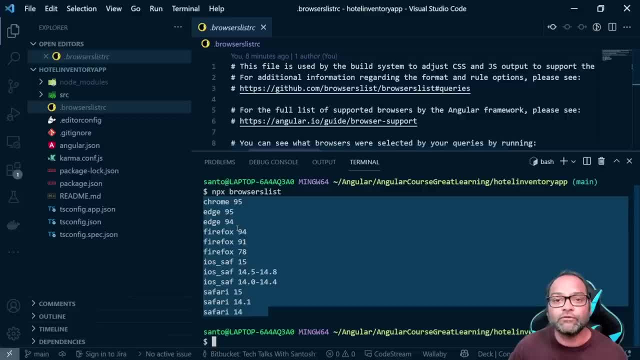 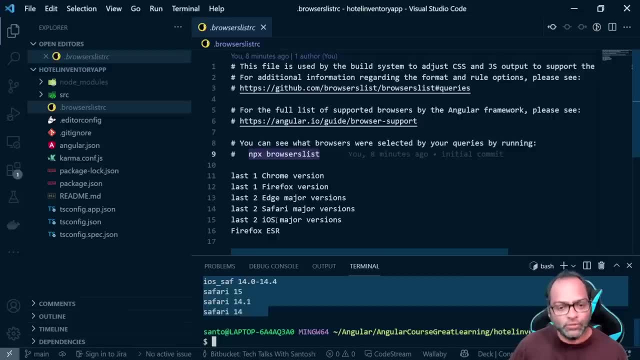 and some other versions. right, so this is. this is the uh browser list which will be generated. if you are wondering where is i11? no, i11 is not supported anymore. has dropped the support for i11.. In case you want to support, just add or remove something from refer to this browser support. 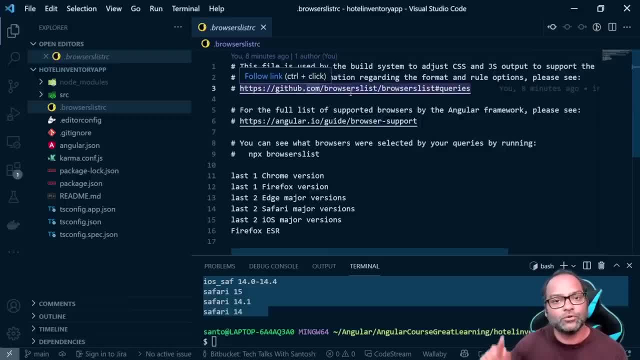 section on angulario, and you can also go to githubcom to see all different browsers, which is available and then what needs to be done to add those browsers here. So this is browser list rc. Now, apart from that, what we have here is src folder. 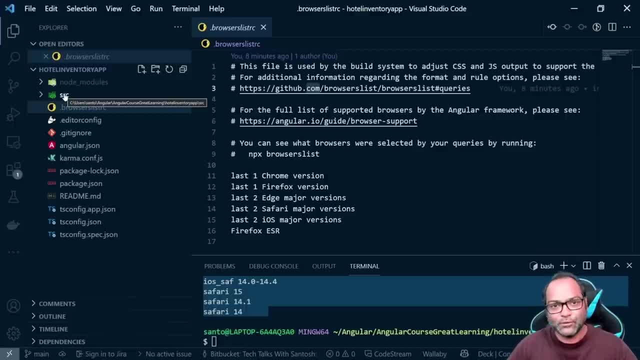 This src folder is where we are going to have fun. It means we are going to write our code here, Node modules. as said, all the packages which is installed will be available in node underscore modules folder and it should not be checked in. So let's see- and now let's go back and talk about src folder- what we have. 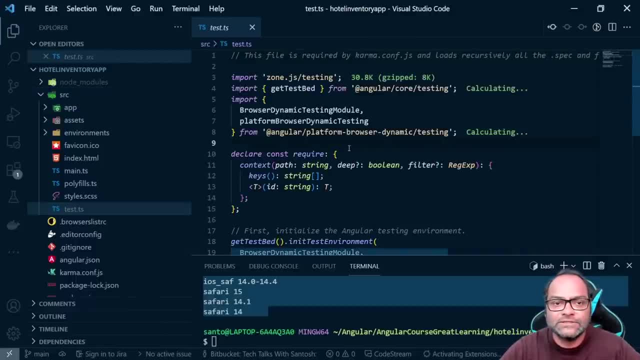 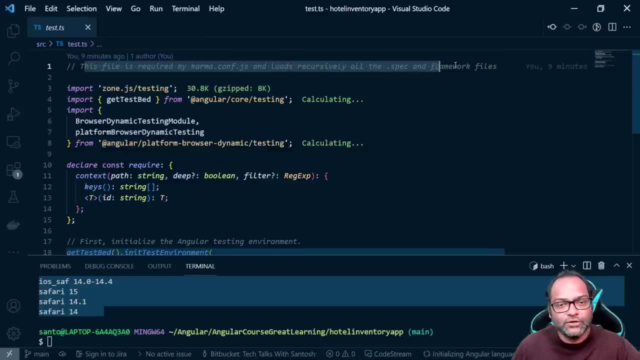 Again, we will start from the bottom. So first file which we have is testts and again, this file is something which, where you don't have to do anything. So this is used by your karmaconfigjs file. It actually just loads all the files recursively, that's it. 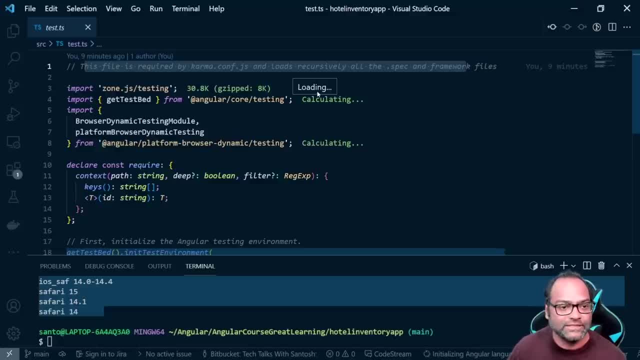 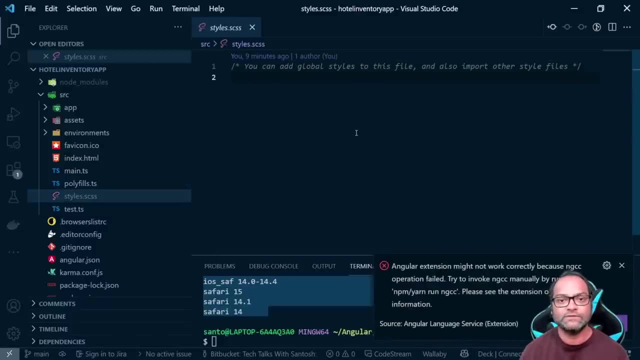 To all the spec files, right? So it loads all those files and give it to karmaconjs. that's it, So you can execute. Then you have stylescss file, which is your global style sheet file. So in case you want to add any global styles, you can actually add it here, stylesscss. 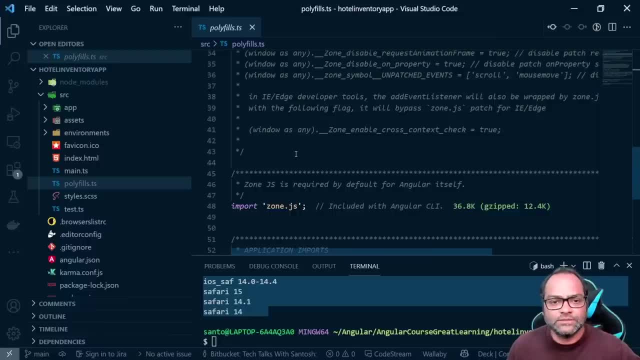 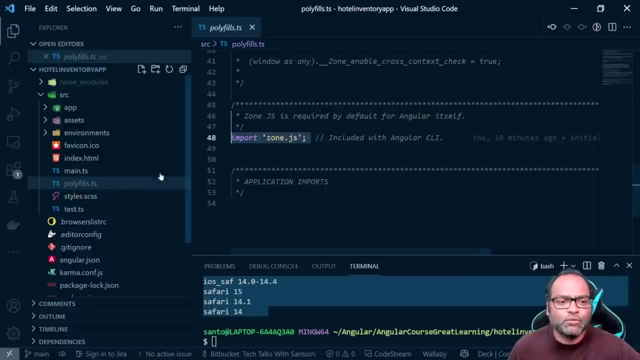 Polyfills, very important file. So you can see something. some, some text is written here And then you have only one import called zonejs. What is this? polyfillts? To understand polyfills, you have to like. we have to talk a little bit about javascript. 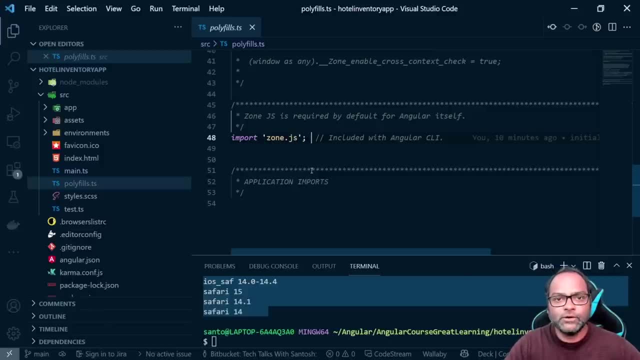 So remember when we were talking about- remember when we were talking about typescript, we said typescript can be compiled down to any version of javascript we need. Does all the browser support all the version of javascript? Probably ES 2017.. Yes, But what in case we have ES 2018 or 2019? even not all the browser supports a free feature. 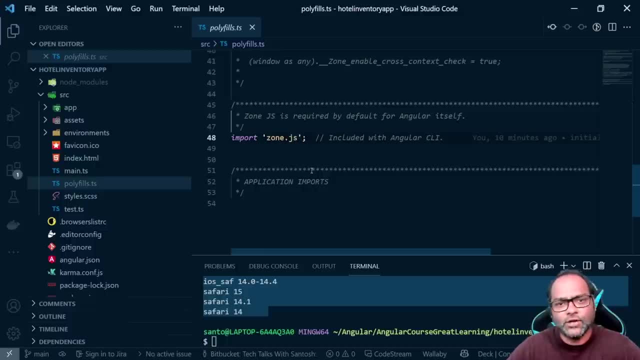 from ES 2015 or ES 2017.. So how to take care of those features? So what you can do is you can add polyfills for those features. So what polyfills does is it will make sure that your code, which you have written, are. 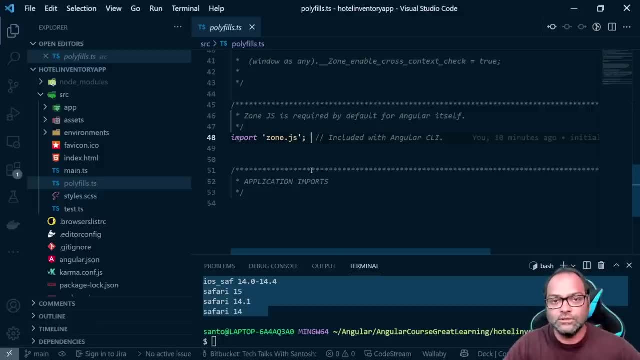 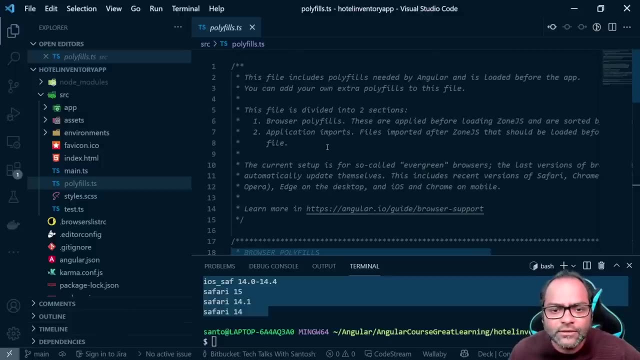 backward compatible with some older browser. So, for example, let's say animations, So one. there is one package. Let me see If I can find it here. Okay, this, that's removed. Now we don't have that anymore. but earlier, in earlier version of angular, there were a. 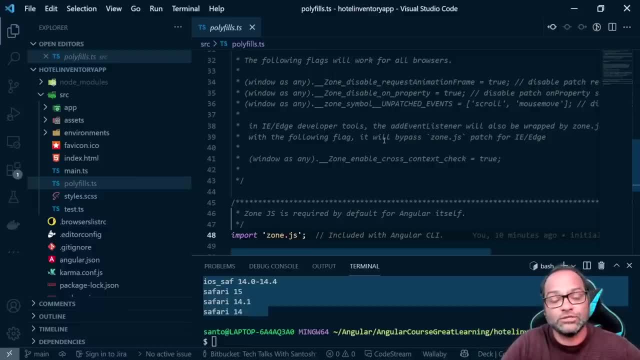 few packages which we need to install in case you want to support animation on i11.. So of course, now i11 support has been dropped, so that is removed, But in case you want to support some features which is not supported on one of the browser. 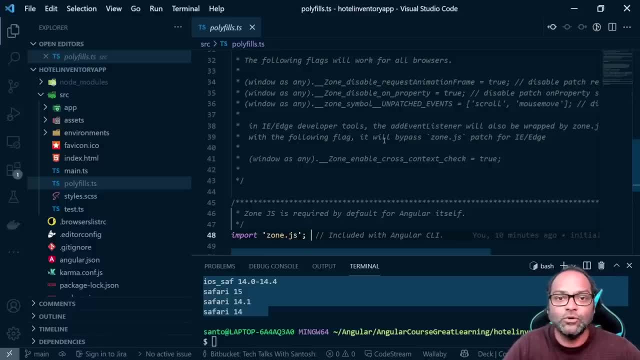 you can add polyfills, So polyfills will just add some extra code. Remember, it will always add some extra code, So it will always add some extra code. So it will always add some extra bundle or extra lines of code to your final bundle. 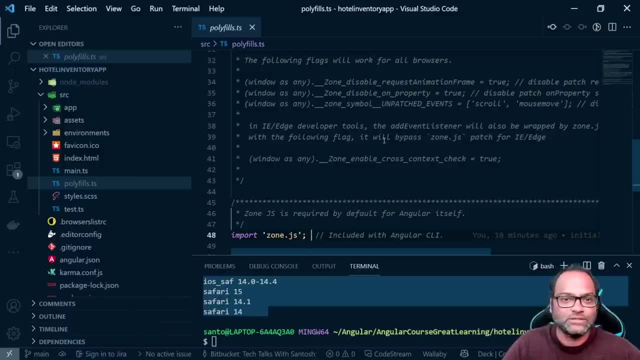 So you may like get some performance- not performance it- but yeah, you may get some larger bundle if you add polyfills. That's. that's the only thing why imports zonejs is here. zonejs is needed to run all the code, which is so zonejs is something which actually patches a lot of features or a lot of code. 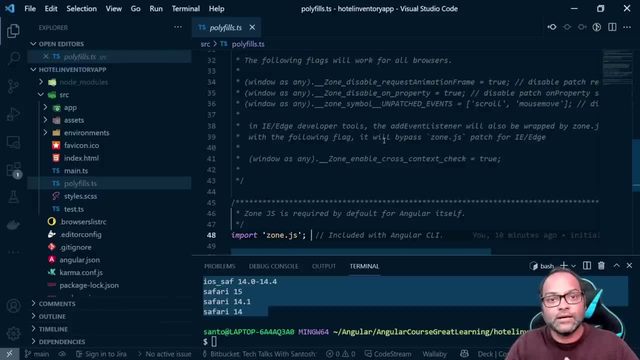 which is not supported by some browsers. Uh, It is used internally by angular. that's it. that's the purpose. in future, angular team is planning to remove zonejs, but that's something which is in which is still in development, So right now we cannot, we cannot remove it. 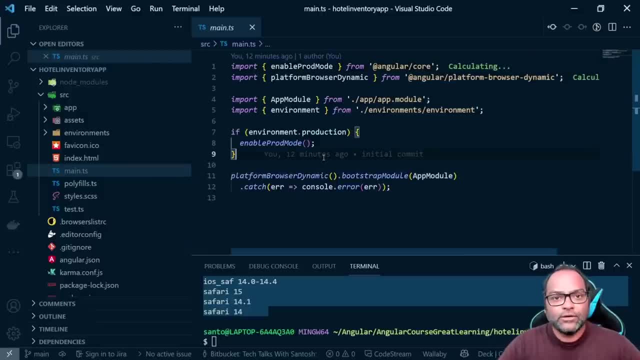 So that's polyfill for us: Maints. what comes in your mind after hearing this file name? maints. of course, in case you are coming from java or any programming background, you may have heard about main, static, public, static, void main. So whenever we talk about main function which says: okay, this is where our execution starts. 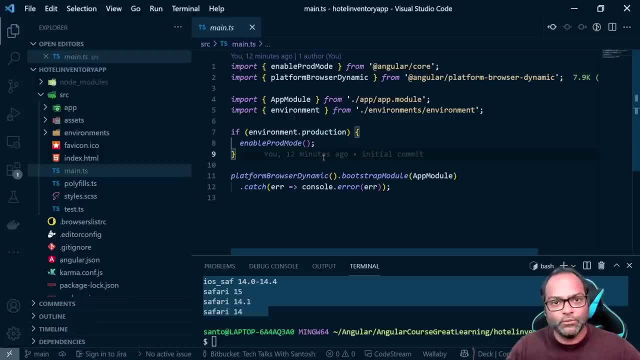 So this is the same file for angular. This maints is entry point, where our application execution starts. So whenever you like create a new application, run it. this is where everything starts. So you have something called. if it is running in production mode, this is environment variables. 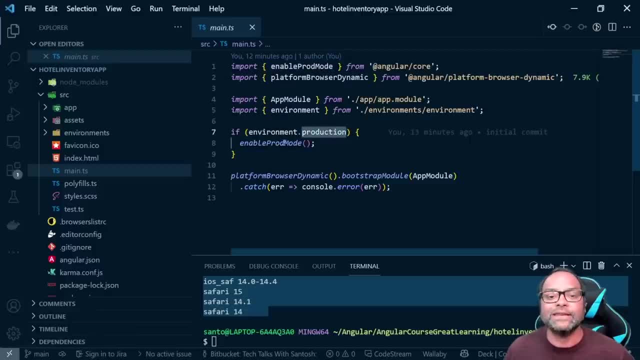 So it says: okay, in case I'm running in production mode, go ahead and enable prod mode. in case we are not, we will run in development mode. So all the development we are going to do and we are going to run everything in development mode, and then, finally, we will create prod bundle which will be deployed on our production. 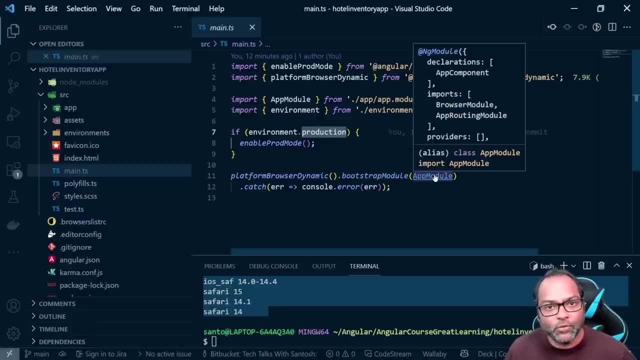 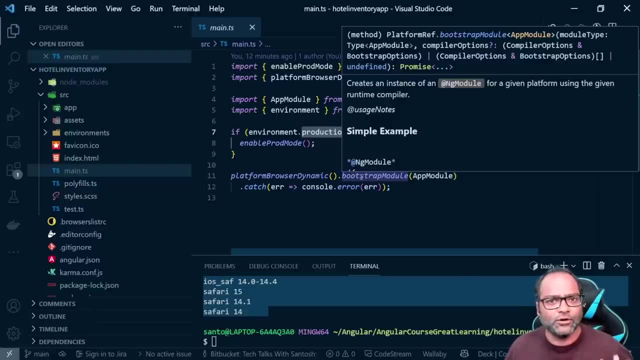 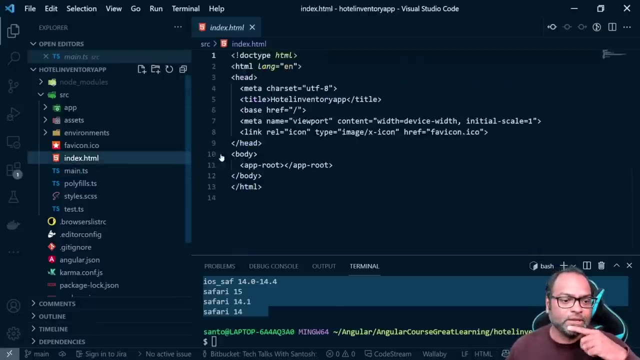 server. Here also we have something called bootstrap app module. we will talk about this in foos in in upcoming section. right now, don't worry about it. the only thing which we want you to understand here is this: maints is our main entry point. Then you have indexhtml, which is our main indexhtml, which will be served. 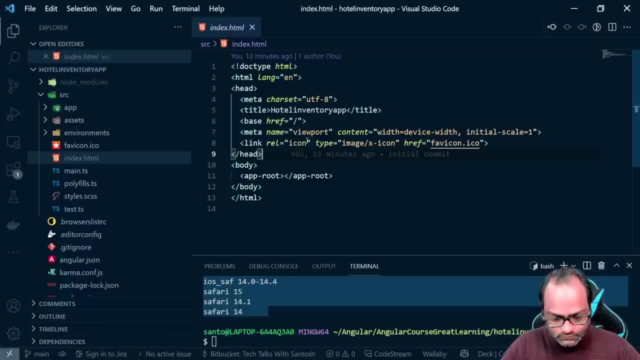 Okay, Remember we said so. this is main indexhtml which will be served to your user. So angular is SPA single page application and I'm sure you- so most of you- are already aware of this concept called SPA because all the frameworks which you use nowadays we talk. 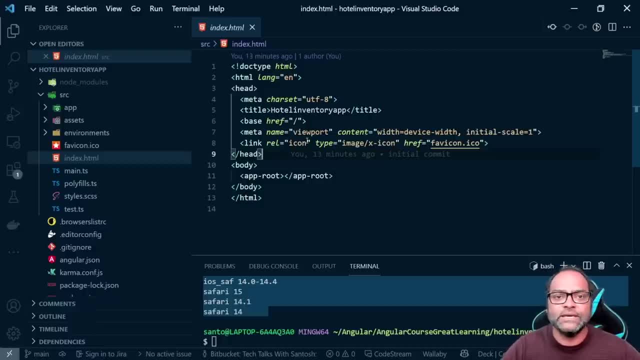 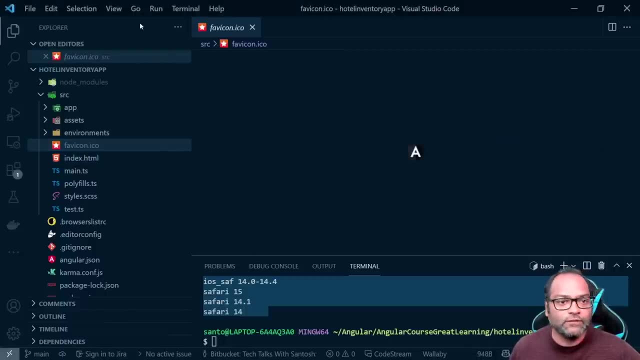 about SPA single page applications. we will talk about SPAs in detail once we go to routing. This is favicon. This is something which you see on all the websites. This icon which is- you can see github icon here, that's favicon. Then you have environments folder where you can actually create your environment variables. 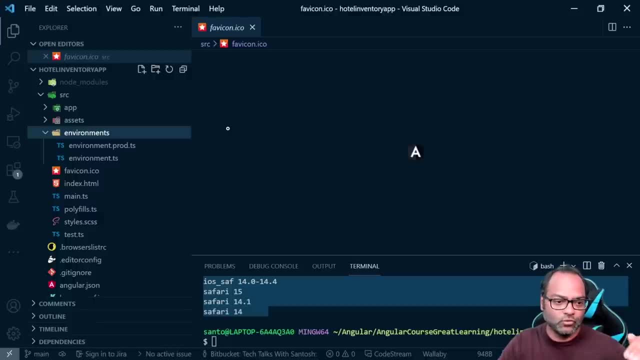 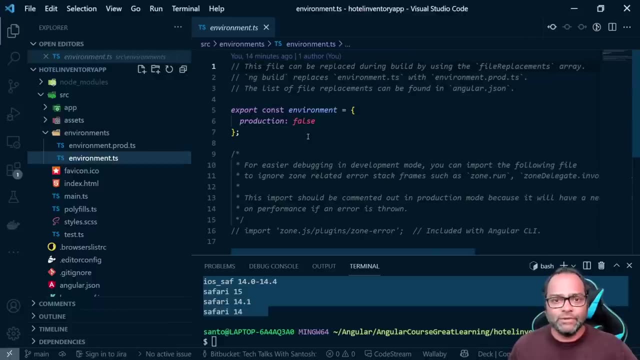 based on different environment you have. So right now there is two environmentts which will be used for development, environmentprodts which will be used for production. We will create some more environment variables in future. just to give you some idea how you can create it. 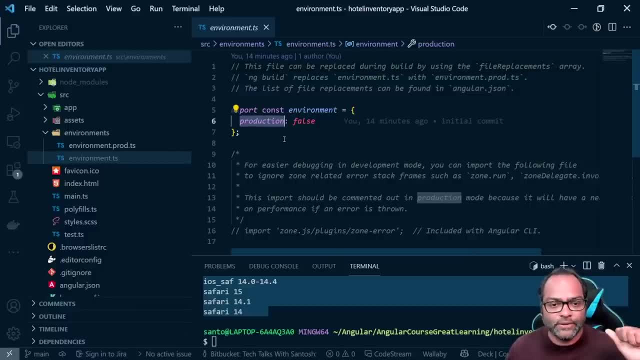 Right now There is only one property called production, So make sure whenever you add more properties, you should add it in both files, otherwise your prod build may fail or any environment variable, environment based file which you have created may fail. Assets: this is where we are going to keep, all keep- our assets. 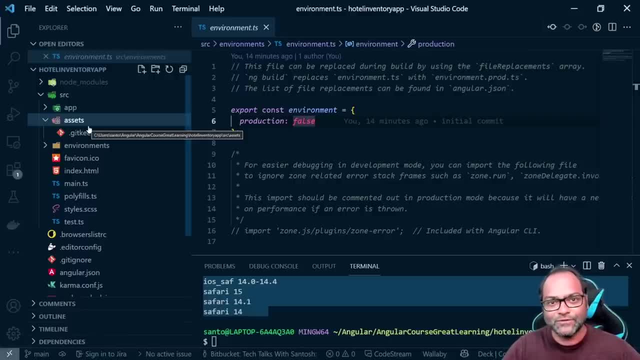 So what is assets in programming, right? So whenever you work with frontend, of course you will have images, some static files. everything goes into assets. So just don't keep it anywhere else. Make sure that you are adding it in assets folder. Then you have app. 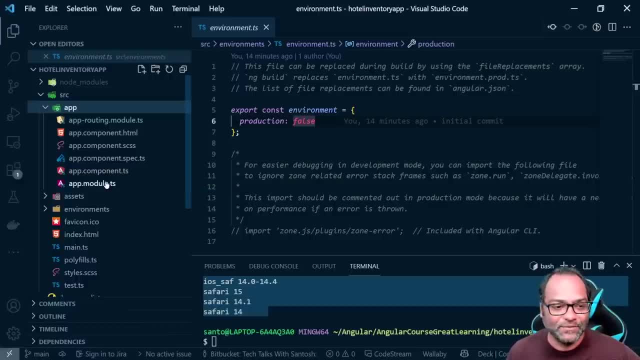 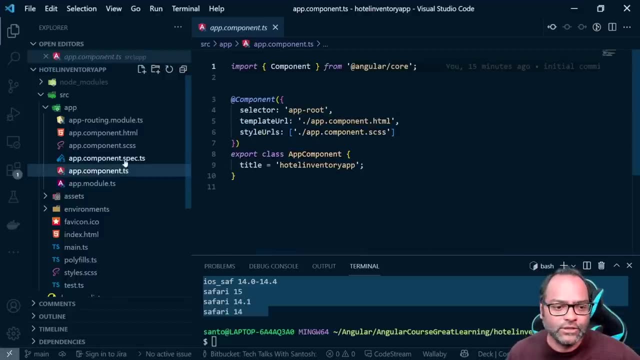 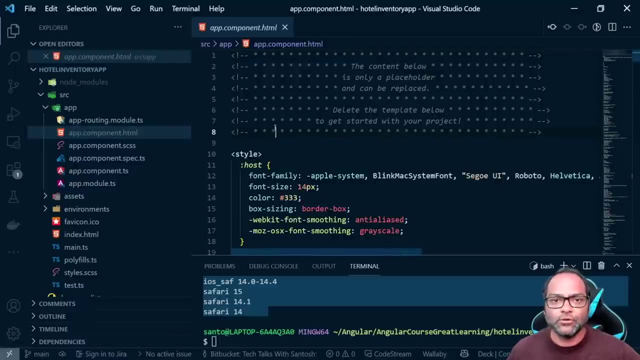 This is now, finally, this is the folder where we are going to write our app. sorry, this is the folder where we are going to write our code. So you have an app module here, componentts, spects, then you have stylesheet file, css file, html. this is where you are going to write your html files, and then you have app routing. 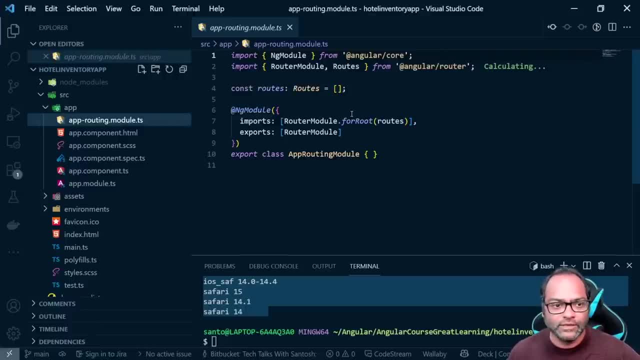 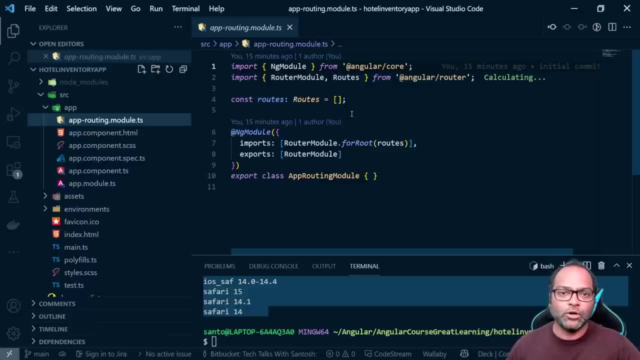 Why this file is here. This is related to routing, So don't worry about right now, we will talk about this file. So when you once you say, do you need routing module, remember the question which we had- do you need a routing module? when you said: say yes, this file will be created and, of course, 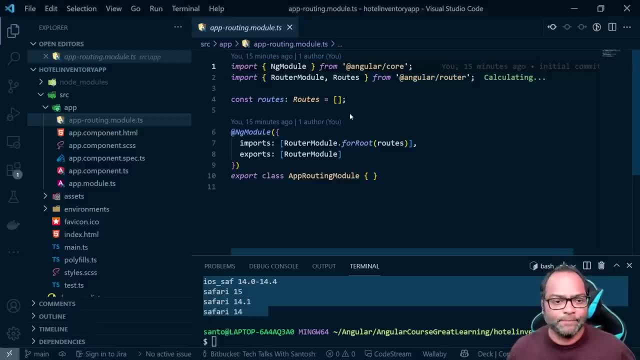 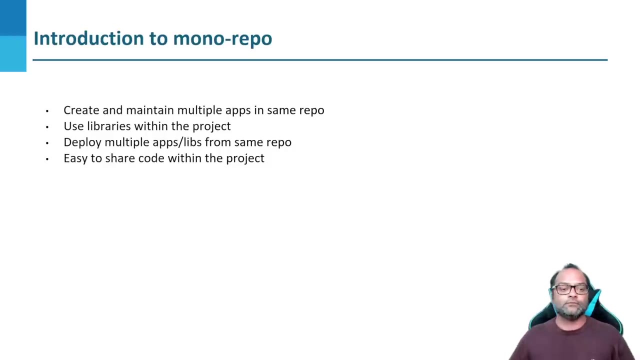 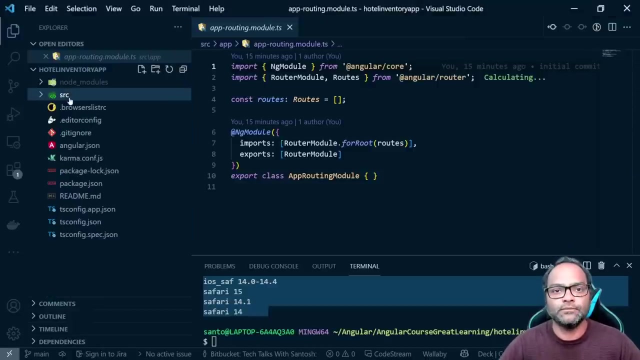 in case you need routing functionality, you should say yes. So these are the files. So you have modules, component and now let's move ahead. Before we go ahead and write our code, or we will talk about this module which is available here, componentts, files which is available here, let's talk about important thing. 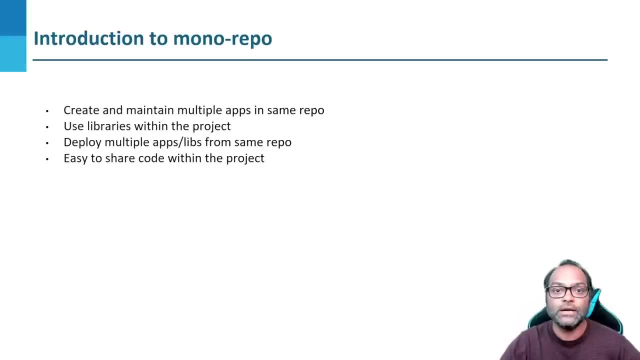 So we said in angular, you can create multiple projects within your workspace. That's something called monorepo. So what is monorepo? so monorepo is something where you can actually have multiple applications. So in angular you by when I say multiple applications, you can have multiple application and libraries. 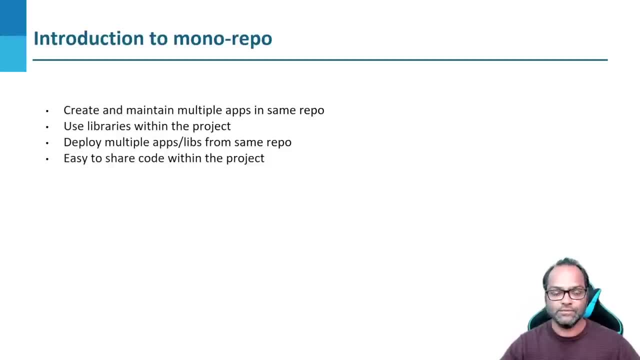 both. You can actually create angular applications as well as libraries, and inside a single workspace You can also deploy multiple applications from your monorepo. That's advantage. For example, Let's say you have A client who has like their admin dashboard and then there they have a client facing in 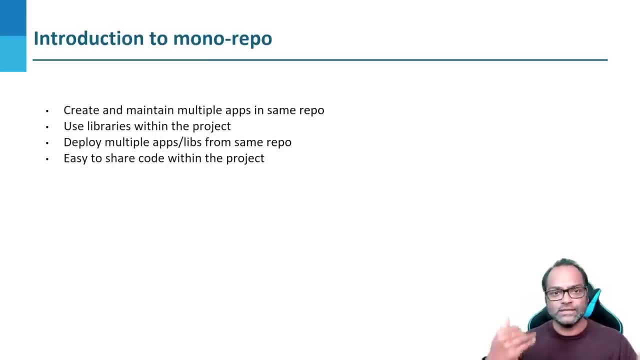 a client facing application. what you can do is you can just have both the application in a single monorepo and you can also create libraries which will like be shared code between or between both the applications, and then you can also deploy both application from the monorepo itself. 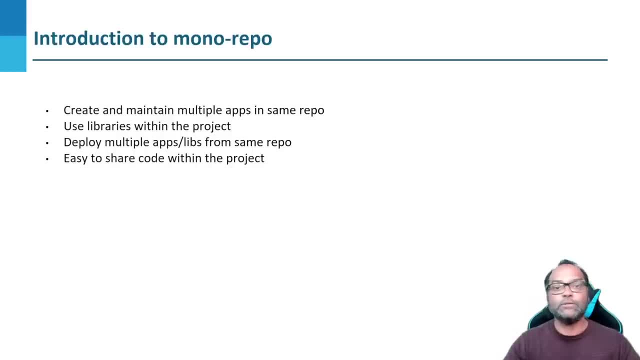 It also makes sharing the code between multiple projects easy. So you Have, like, a separate team which is working on admin application, a separate team which is working on your client facing application or public facing application. What they can do is they can create like: extract the common codes, keep it in library, share. 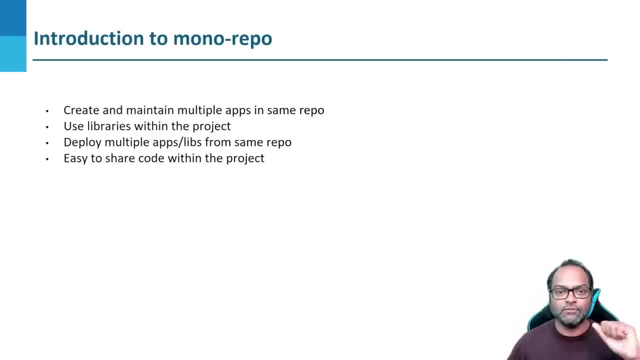 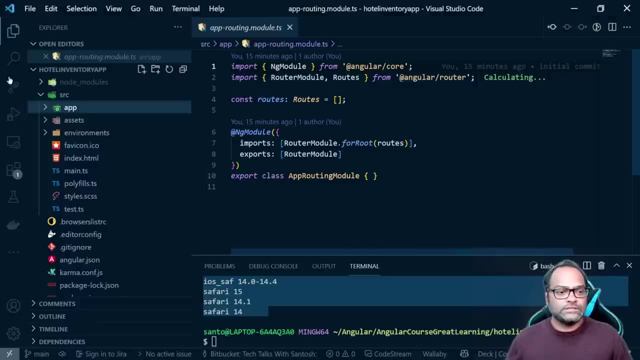 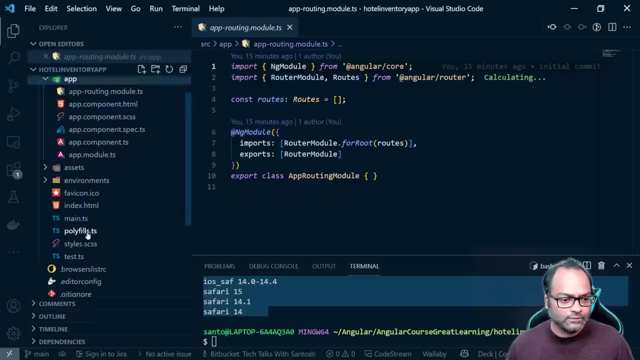 it across and then use it saves a lot of effort, a lot of time and it makes, like, collaboration between multiple teams much easier. So this is it from here: The workspace and monorepo. Now Let's talk about few things, few files again, maints and other files. 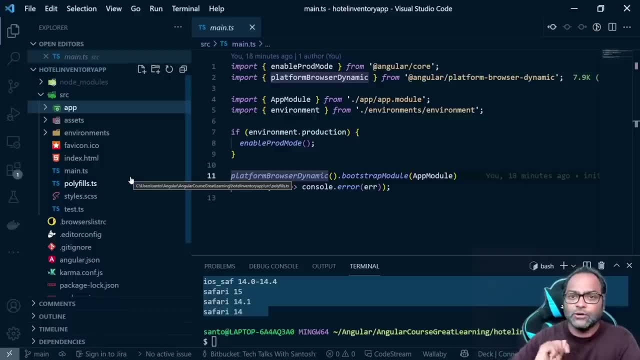 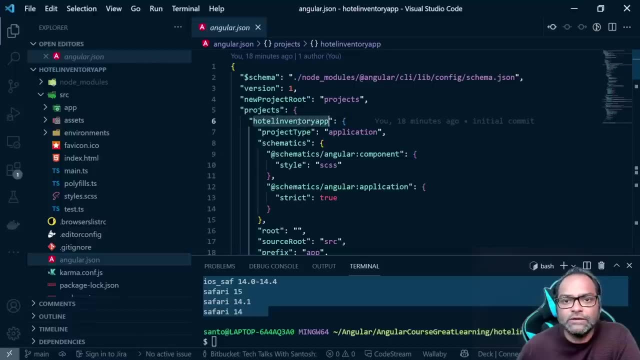 I'll show you the connection between this files and your angularjson file, how they are connected. So let's go to angularjson file and this is our project right now: hotel inventory app. It has project type, So this is how you can identify if a project is library or application. 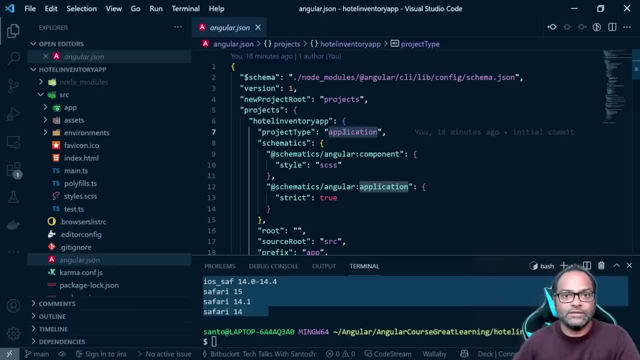 Application is, of course, your application which can be deployed somewhere and then Which has, like your visual visuals, or front end application kind of thing. So that's application library, something which is which will have your reusable codes and you can use those libraries, build those, use it or publish it on nbm. 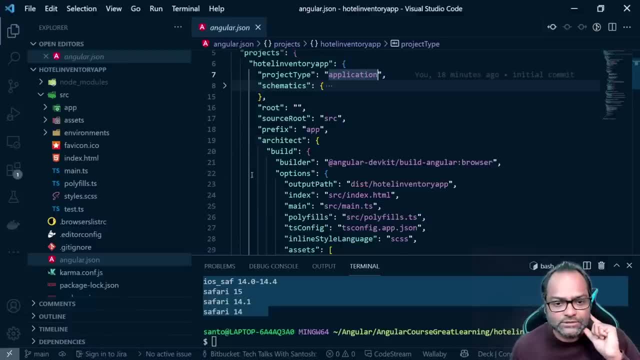 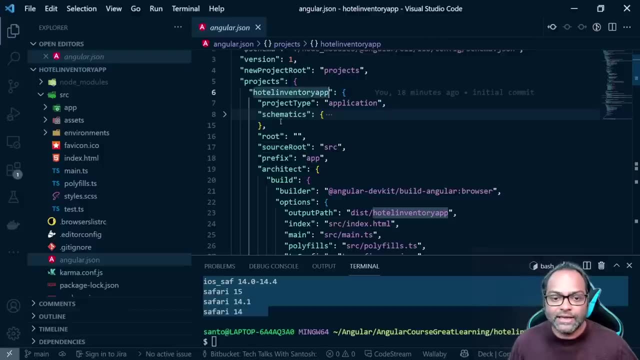 Those are libraries, So let's go ahead and see. So there are few properties. So first this hotel inventory app. What is the source root for this application? So it says SRC. So this is: This is the folder in case we create a new application. we will see that later on you. 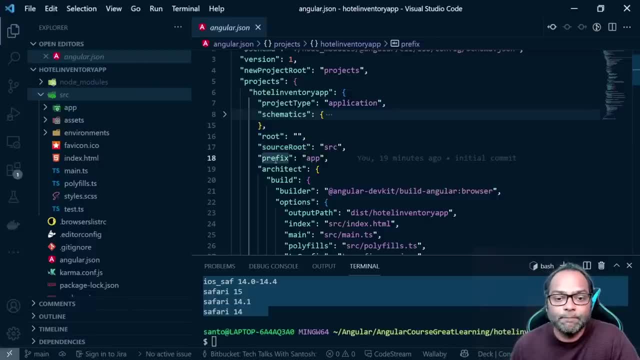 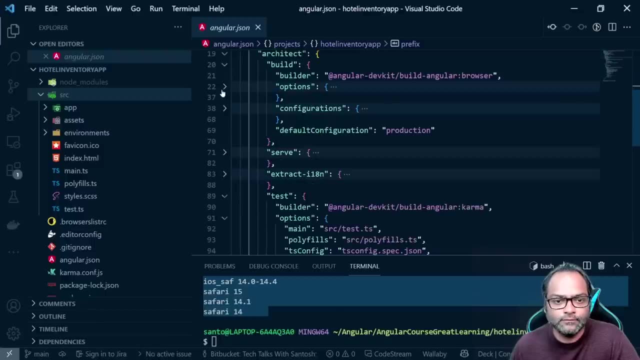 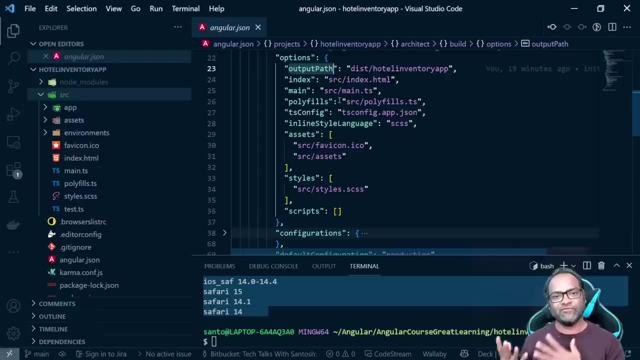 will see. the source root will be a different. folder prefix will come back to this. Before that, let's see some more options. So here, the first property which you have is output path. This is where all the final bundles or final code to be deployed will be created. 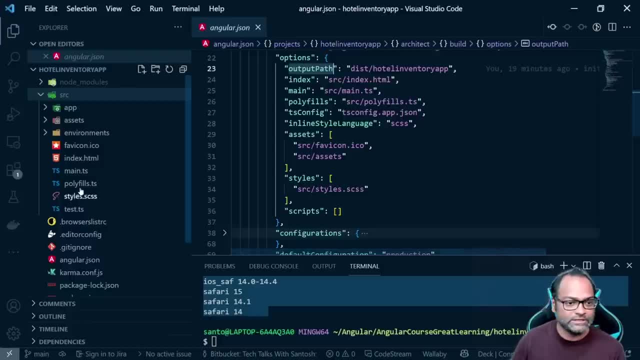 We'll talk about this. then you have index file. So remember, We said, OK, this is the default indexhtml which will be served to the consumer. Does it need to be indexhtml? The answer is no. You can name it whatever you want, but mapping should be here. 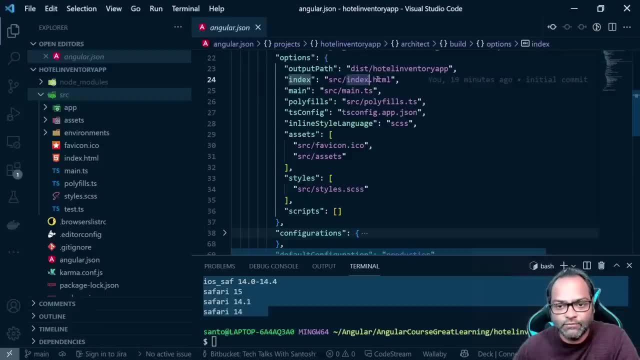 So you have index, which will, which have a path to indexhtml. So this file, similarly main maints again. So this is referring to this file, So it can be any file name. I'm just saying, OK, this is the mapping, this is how they are mapped once you start building. 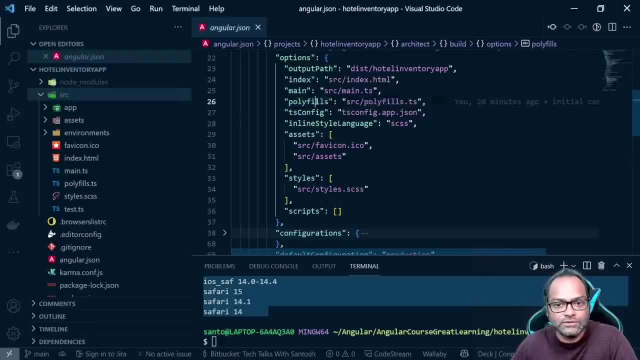 your application, Then polyfills, of course it is defined here. So, in case you want to add, You want to have a common polyfill. for let's say, you have a monorepo with 10 applications. Now do I need to actually have multiple polyfillsts? the answer is no. you can actually go ahead. 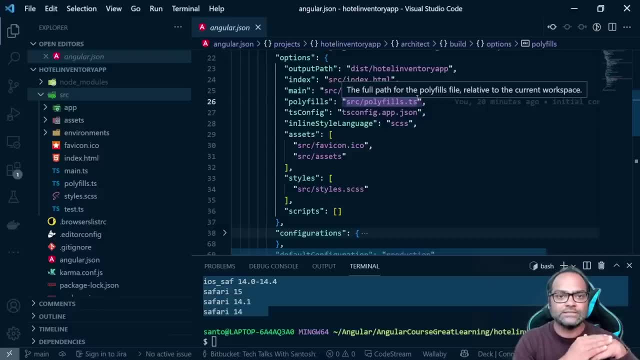 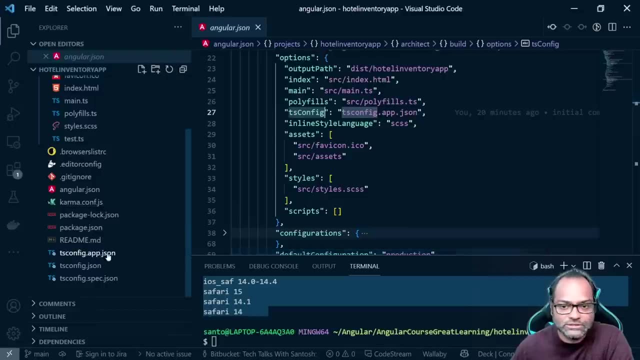 and just create a polyfillts somewhere in a common folder and then use it. That's possible. tsconfig, as we mentioned, for app tsconfigappjson will be used and there is a new property called inline style language. You can Here writing: inline sass was not supported nowadays. 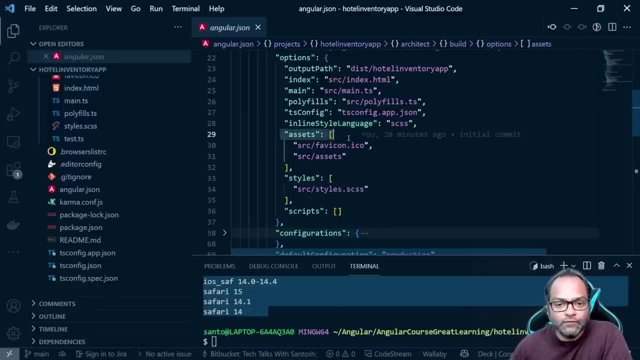 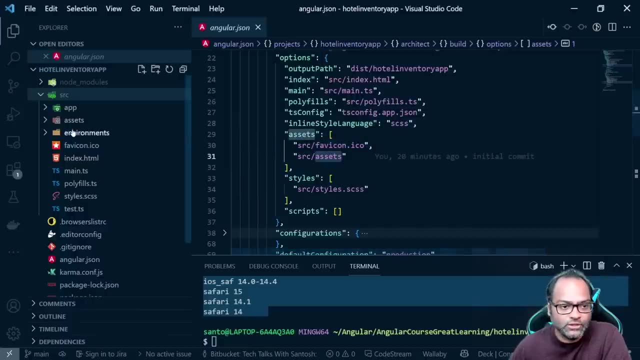 So that's, this is the property which is used And what will be actually available inside your assets folder. So you have favicon and the assets folder. So once you, let's say, keep some images in your- let's say- separate folder, right, Generally try to move them into assets folder. 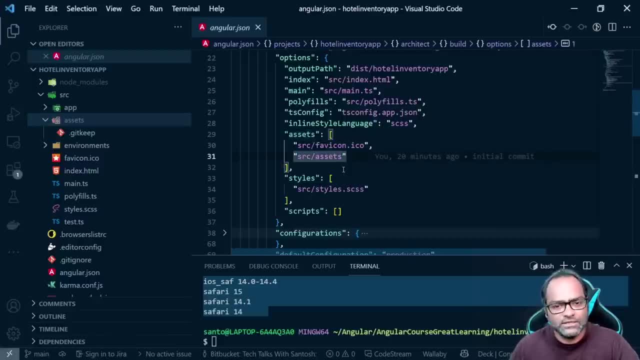 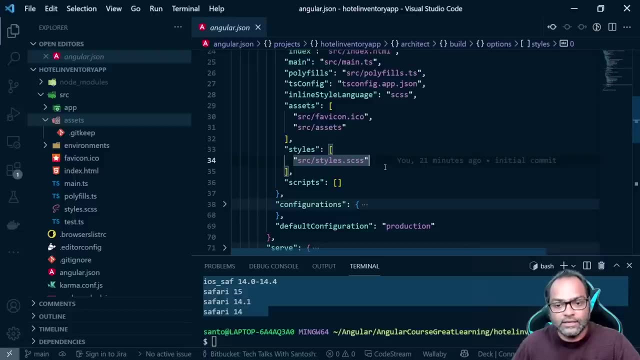 But in case you are keeping it somewhere, you can actually pass a path here. stylescss, This is your global styling, global stylecss, And in case you want to include more styles, you can actually mention it here. for example, let's say you want to add bootstrap, you want to use angular material, you can apply or add. 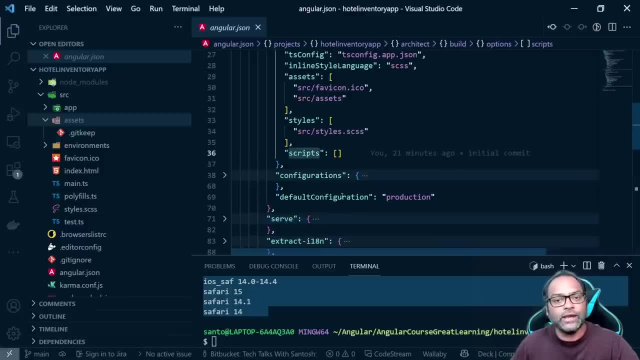 all those parts here, The scripts. you can actually load some js files as well. So you can actually give path here, in case you have some requirement to load some external javascript, otherwise just don't. So these are the files which is related. Now let's go back to maints. 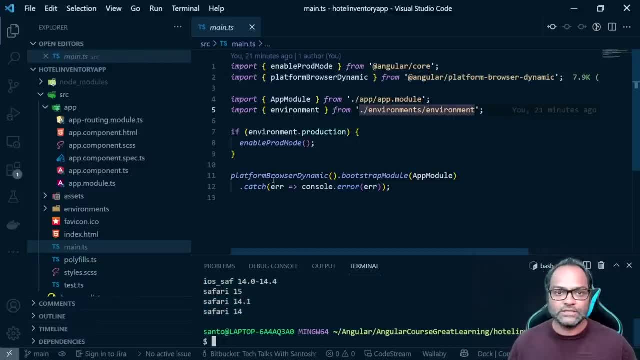 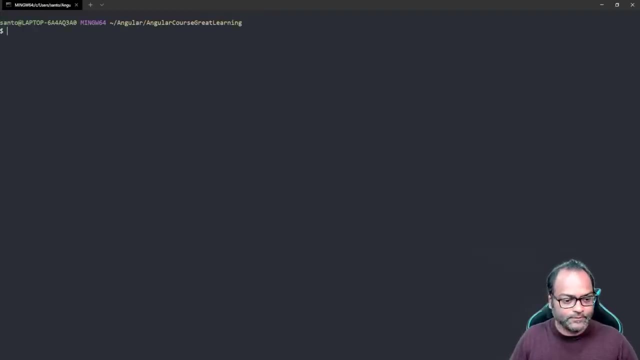 So here you have your maints and let's run this application and then we'll see the flow, how it actually goes to this, What is this module, and then how you get your first page. So to do that, I'll just open: Okay. 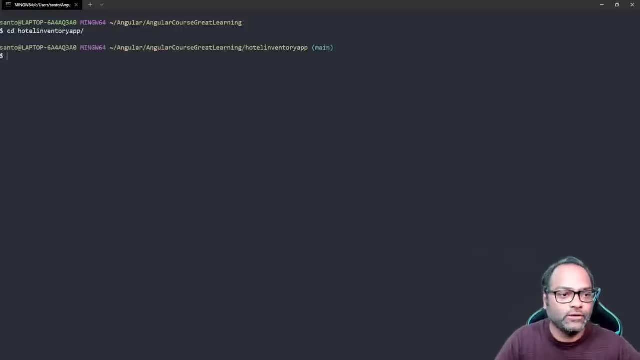 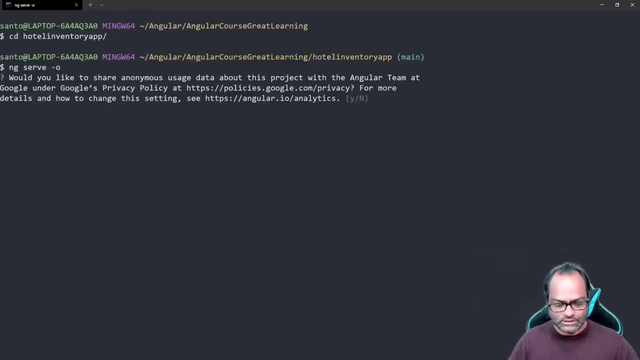 Okay, Okay, Okay. So we go inside hotel inventory app. let me just zoom in a little bit Now. here you have to run a command called ng-src-o to run this application locally. So I'll say I don't want to actually share this information. it's up to you. 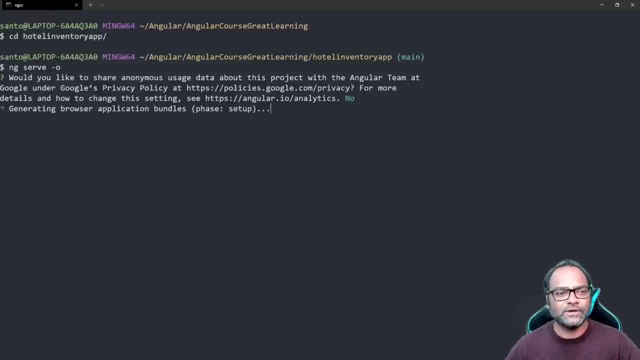 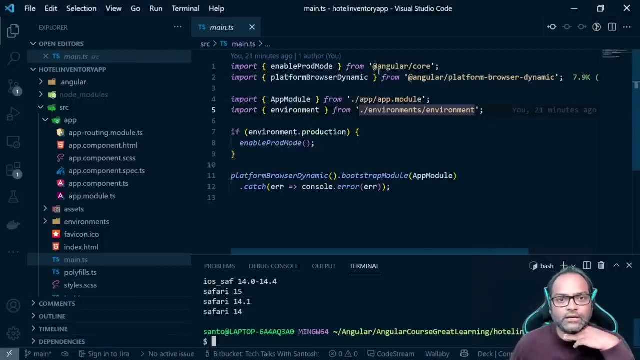 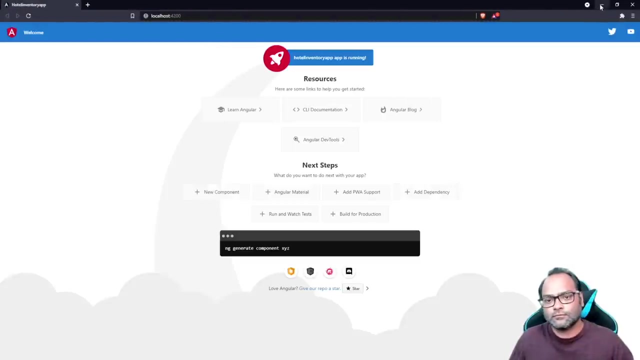 You can just change it to yes if you are working on some side project. So meanwhile it is getting compiled. let's go back here. So here, as we said. so this is your main entry point to the application and it goes to, So it goes to this bootstrap module. 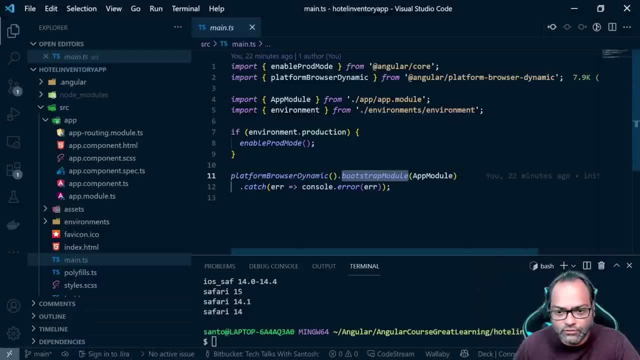 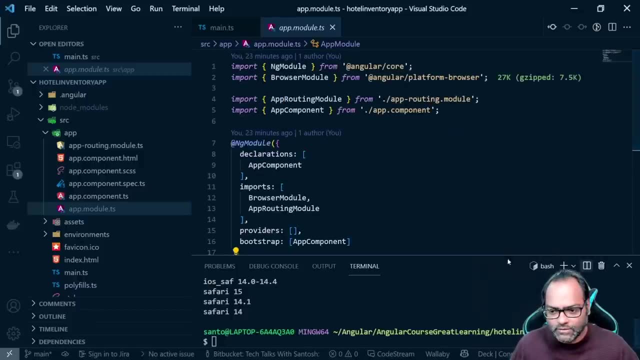 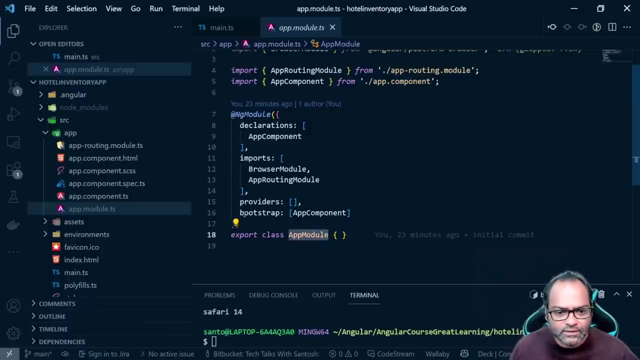 So whenever you use your maints executes, it goes to this bootstrap module and it bootstraps and module which is app module, And let's see what is available here. and it has something called app module class actually, and then on top of app module there is something called at the rate ng module. 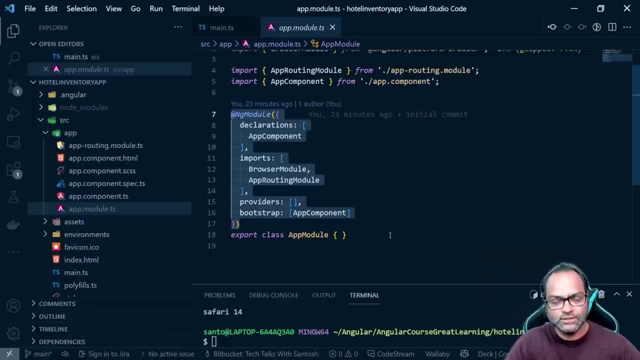 So what is this? let's talk about this and then we will move on to next topic. In angular, everything is a class, right? so you can see this app module. it's a class component, it's a class. But to bootstrap your application you need a minimum one module. remember this. 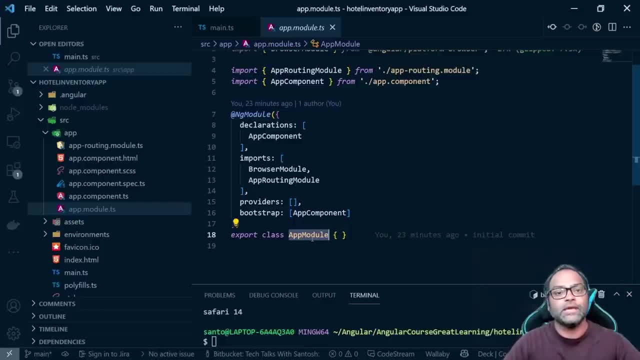 So in angular we call this as a root module. In future it may be possible that you don't need modules anymore, but right now we need modules. what we do using module- we will also talk about that. So right now let's talk about this. 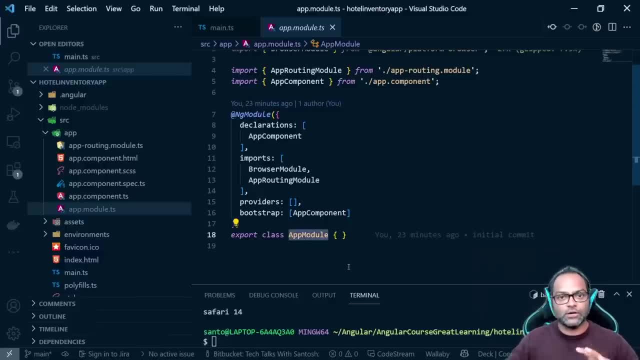 So this class, this is your root module, which will actually have information about all the components which will be created. What is component? yes, we will talk about that as well. It will also contain the information of any third party library or any angular specific library which is being used. 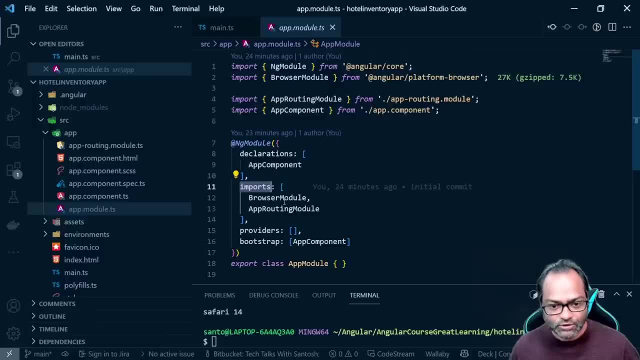 So if you see this import section, it has something called browser module and app routing module. So this browser module is actually an angular module which is available as part of angular slash platform browser library, and app routing module is created by us when we started our, when we created our app module. 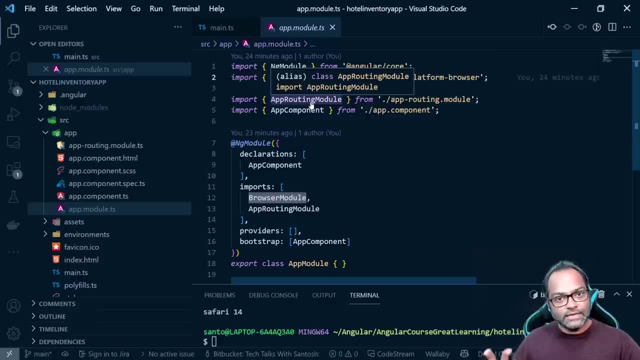 Okay, When we created our application. So when any angular module which needs to be used needs to be imported into imports array, any components, directive and pipes. remember these three words. we will talk about all these three. any component directives and pipes needs to be registered by declarations. 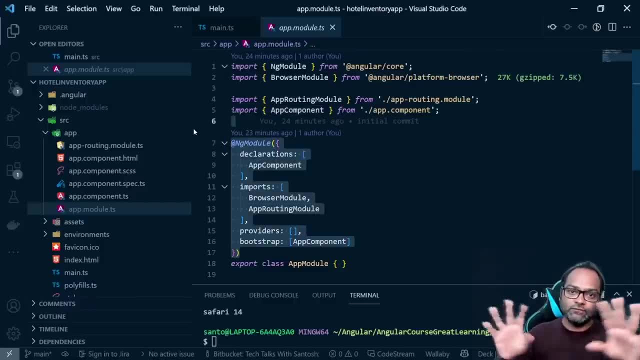 array and this ng module will have all the information about different components, different angular modules, which is being used or any module which you have, You have created by your own. it means I can have any number of modules, I can create any number of modules in my application, but it needs at least one root module and that's. 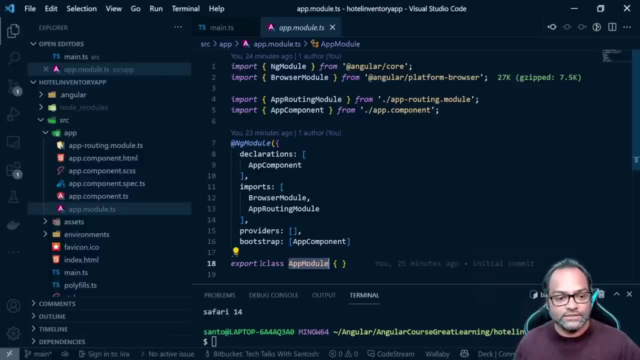 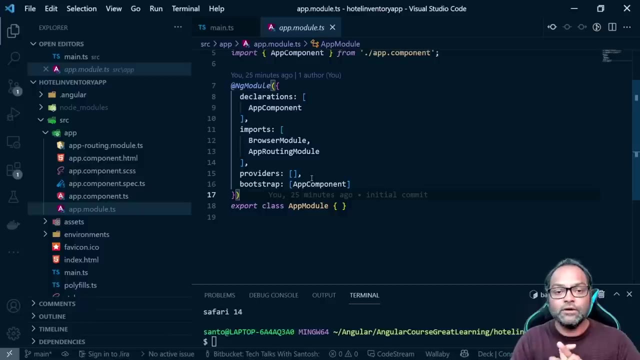 why angular creates one by default and this will be loaded once you start your application or once you build your application. So this is from where your execution starts. So now it gets, goes to app module. app module knows everything about my application. it knows what are the different components. 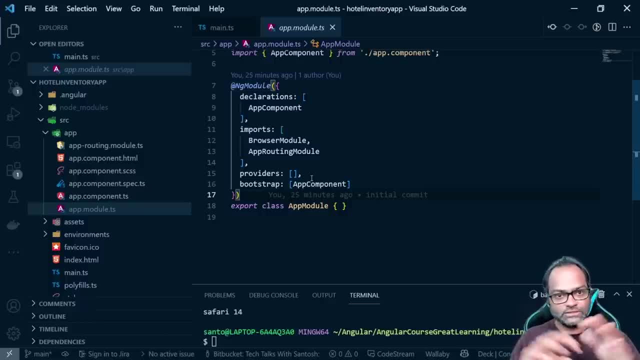 What are different modules I'm using, and it gives that information to your compiler. Now, after this, let's go ahead and talk about this at the rate ng module. Now, your compiler needs to know that, whatever class I'm actually compiling, what type of class is that? what is this? at the rate ng module? remember, just in TypeScript, we discussed 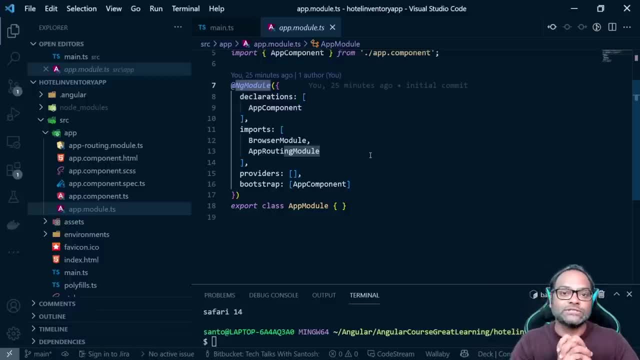 something about decorators. so, and we mentioned that angular uses a lot of decorators, so this at the rate ng module is a decorator. So what decorator does? it? modifies the behavior of your class. So what this at the rate ng module is doing here? It is giving all this metadata information. that, okay. what are the different components? 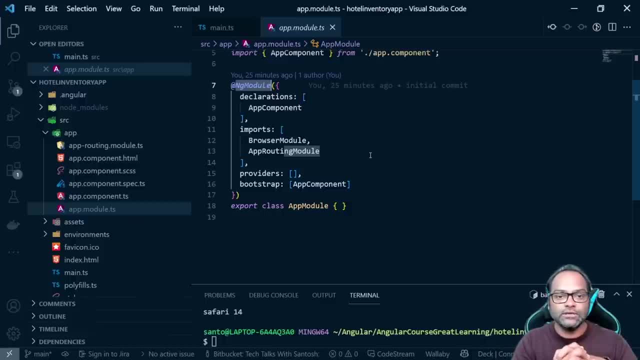 I'm using? what are the different modules, angular modules I'm using to the compiler. Then you have something called bootstrap app component. So now, once you compile all the files, your angular application needs to know that. okay, which component Will be loaded to the compiler? 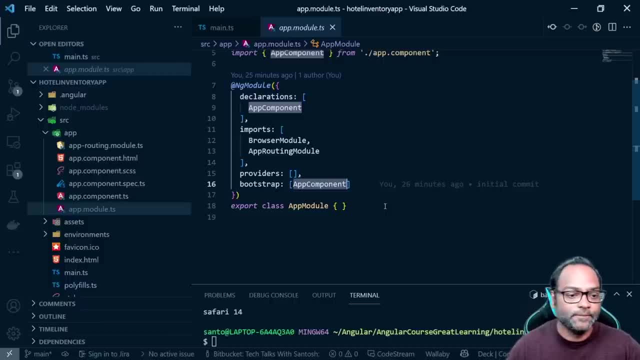 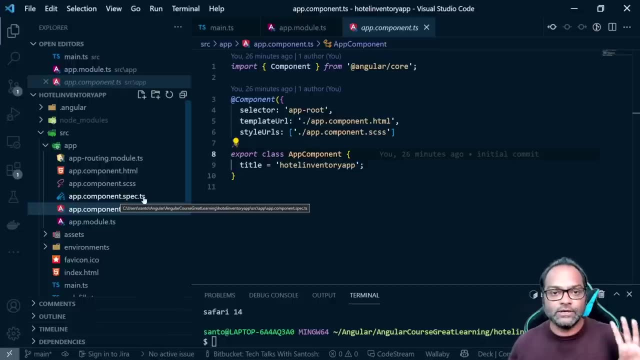 But first, what is component? now let's go ahead and talk about what is component. So it goes to this: app componentts, right, So you can see app componentts. and whenever you create a component, you will get four files. So let's talk about those four files. 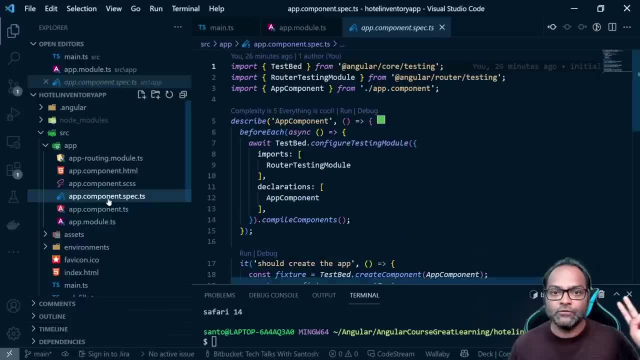 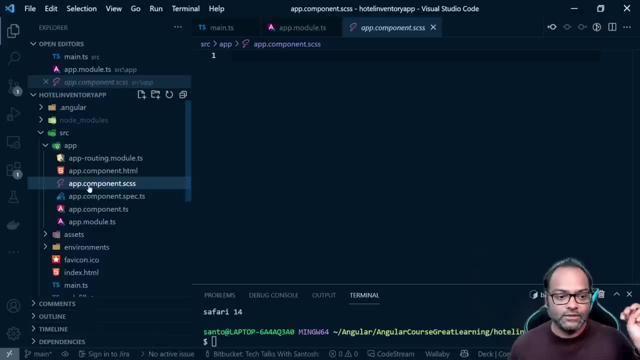 So you will get a ts file. you will get a spects file where you will write your unit test. you will get a css file, or css file or whatever type style sheet you have selected. third, and you will get an html file, your, where you can write your html code. 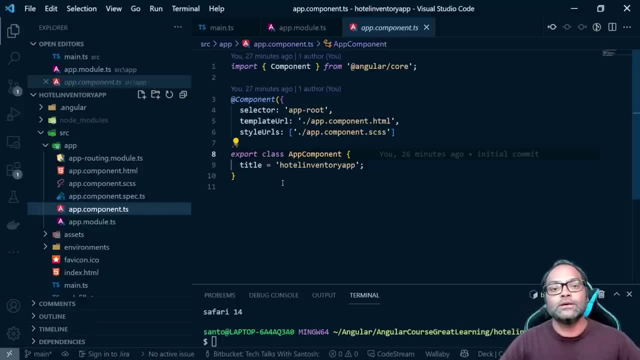 So these four files will be created. Now, coming to component. So components are actually your views which will be actually rendered to the end user. So here, this is my first component, So, similar to my root module, which is, we said, app module, we will have one root component. 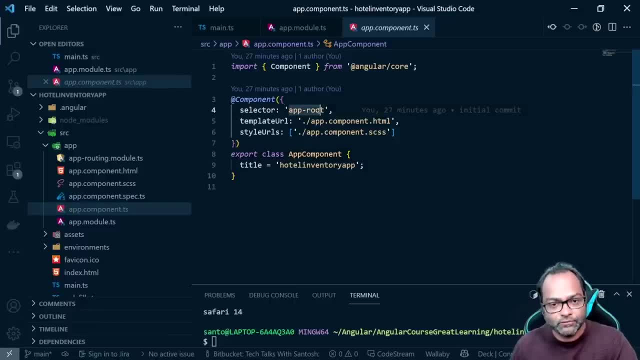 This is our root component. That's why also the selector is named as approot. we will talk about what this selector means and what that template you are in cellular is, but that's why they are. it is named mention as as root, Because we need a root component as well. 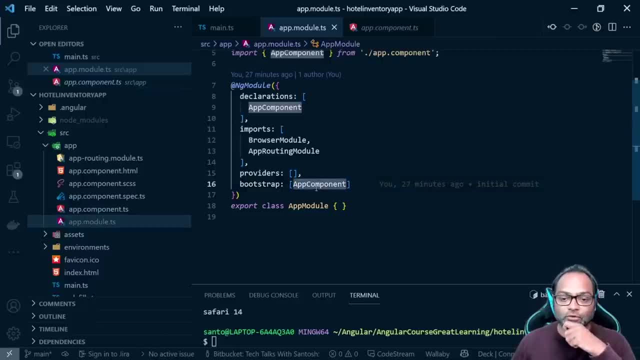 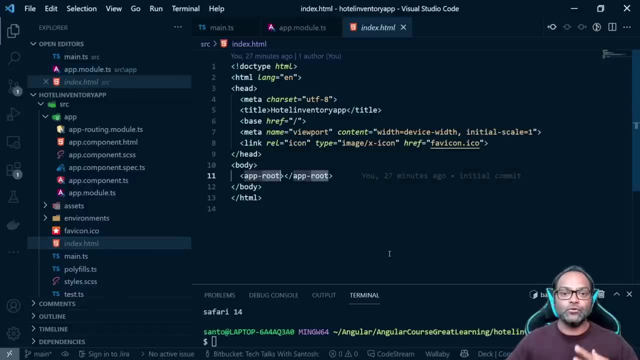 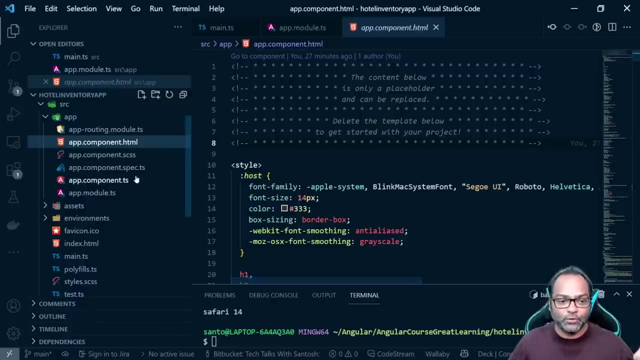 Now let's come back here. So bootstrap, we have mentioned that. okay, this is my root component and this root component will be loaded on your indexhtml. It means, in case I want to load any other view or any other component in future where I can load it, I can load it within this app componentts. 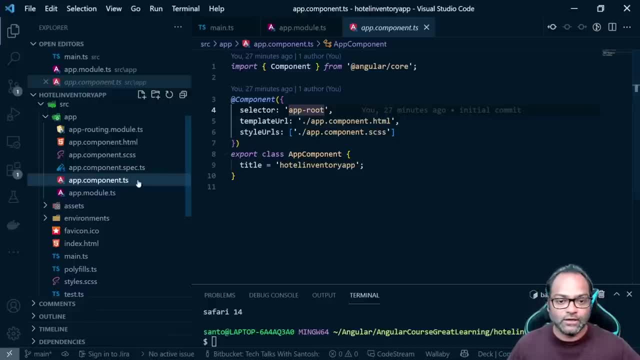 So now let's talk about all other files. So now we are aware that, okay, this component, this is the component of view Which will be available for us now, and these are the four files. So html is where we will be writing our, our html code and, in case you create new components, 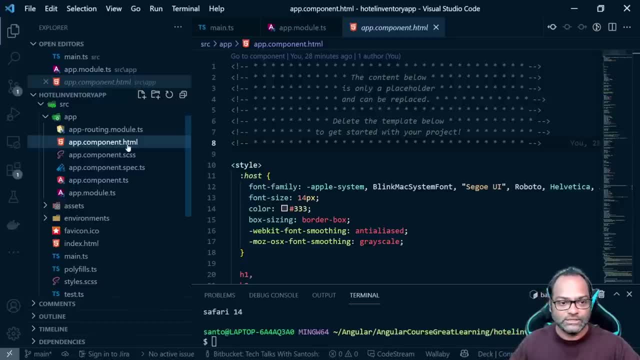 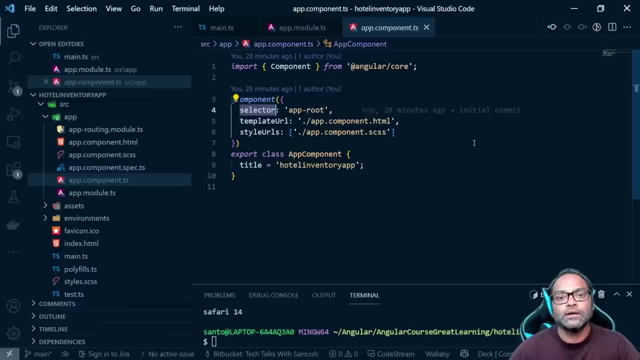 and it needs to be rendered. you will add that into app componenthtml. Let's talk about these properties first. So we have this first property, which is named as selector. So when you create component, actually what you do is you create a view How it will be rendered. 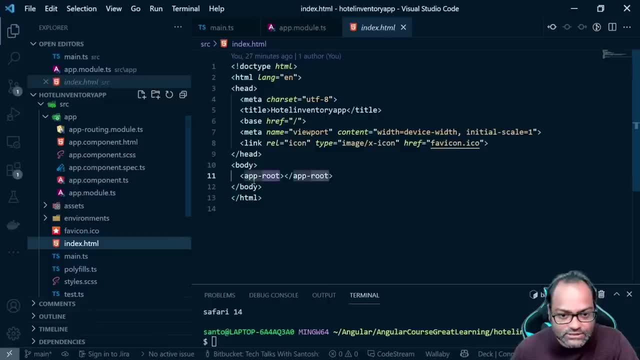 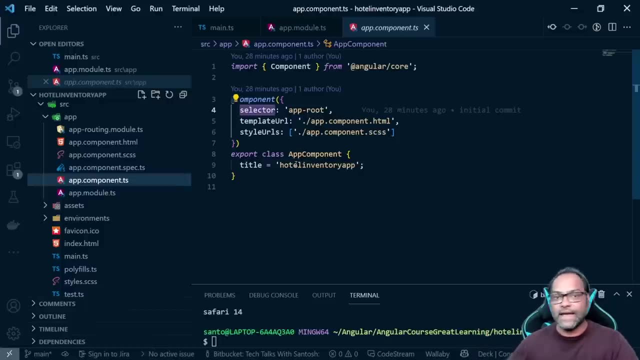 It will be rendered using an html tag. If you go to indexhtml, You will see that This is your html tag and that's what you will be creating. So you will be creating multiple reusable html tags which I can go ahead and use anywhere. 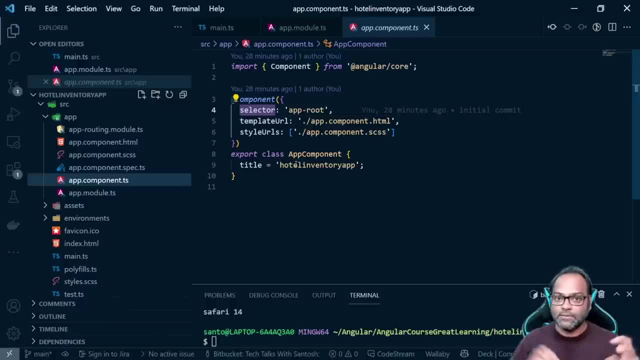 I want to. Those are components, So you go to any library or any framework, UI framework. they will give you this custom html tags, But this is what you will be creating. You will be creating those custom html tags and then you can render it anywhere you want. 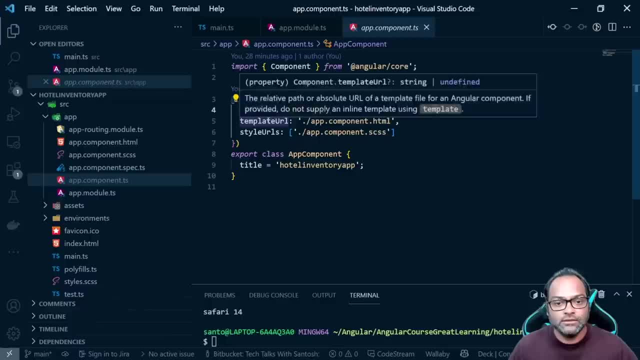 to So here the selector becomes your html tag. Then of course it needs to render some html. So you can do it in two ways. in angular You can either have a separate html file, separate where you can write your html, or you can also. 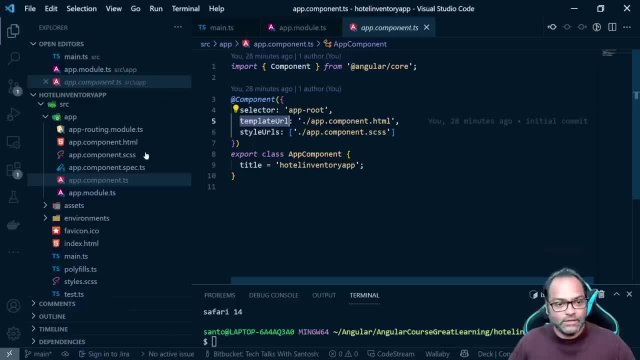 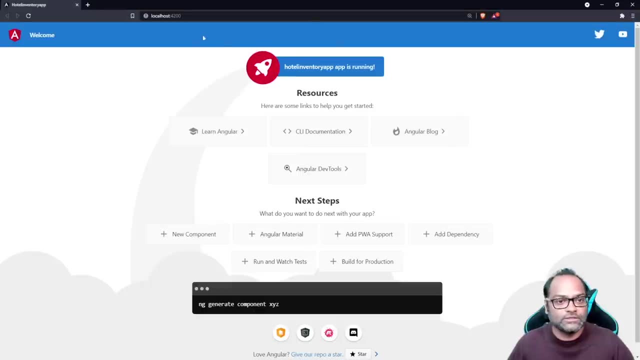 use inline html as well, So this template URL now points to this html. It says: okay, whatever html is rendered right now, it's coming from this html. So if I go to this localhost- 4.2.0.0, all this information is actually available here. 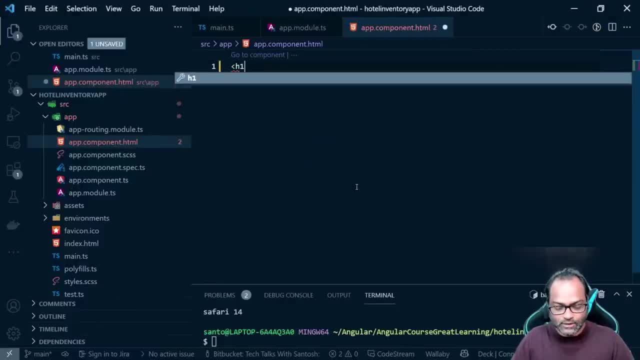 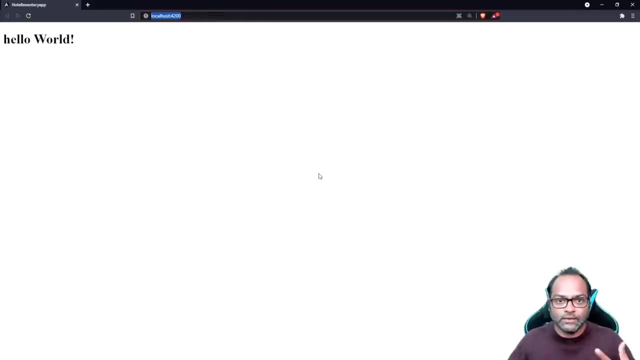 So let's remove it and I'll create an h1.. I'll say hello, Hello, Hello. Thank you, Hello, Hello, Hello, And you can see as soon as I press save. this will be automatically compiled In angular. the ng serve command runs in watch mode. 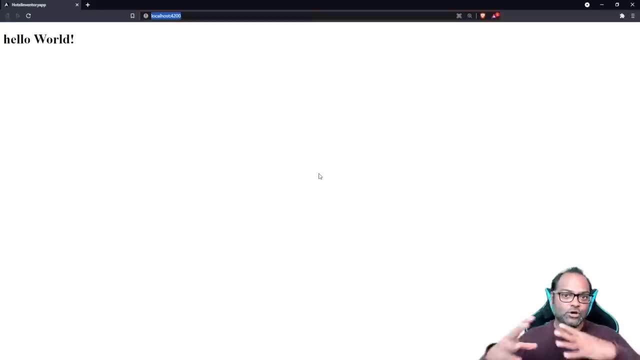 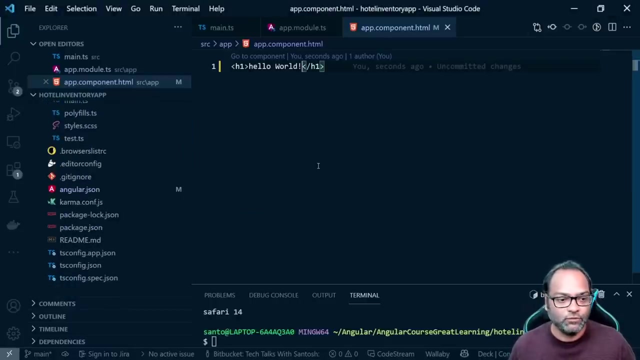 What I mean by watch mode. it keeps and watch on all the changes which you make on your file system or in your workspace. everything is washed. so let's say, if I make some changes to angularjson or packagejson, it won't be actually washed. you make any changes inside your src folder, most of them will be washed and 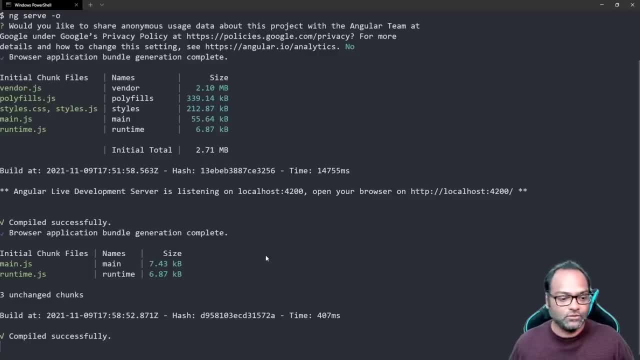 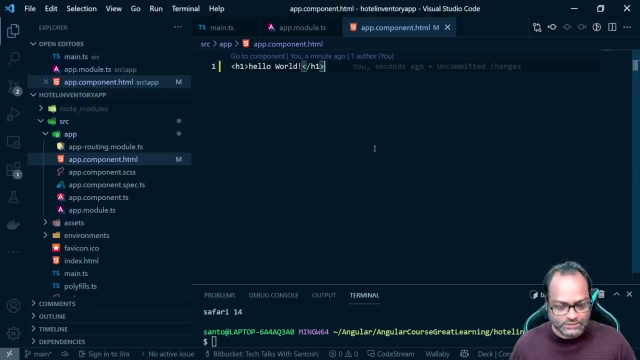 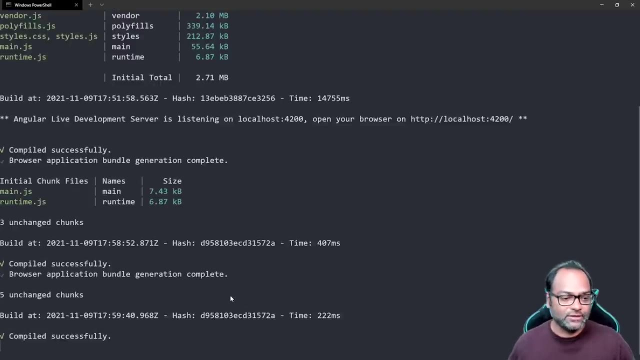 it will just restart the server which is running here so you can see: let's press ctrl s and you can see compile successfully. because of course there were- there were not any changes, so it was so fast that we didn't even realize. but it says: okay, the build time was this. 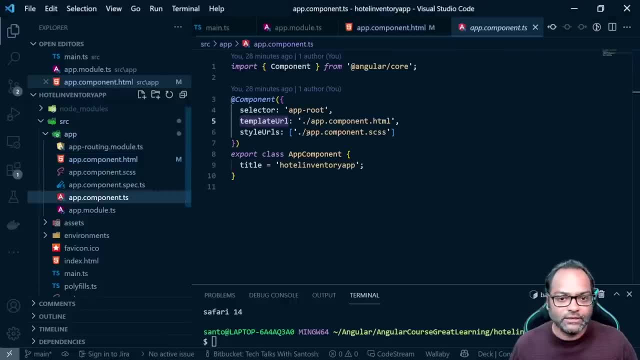 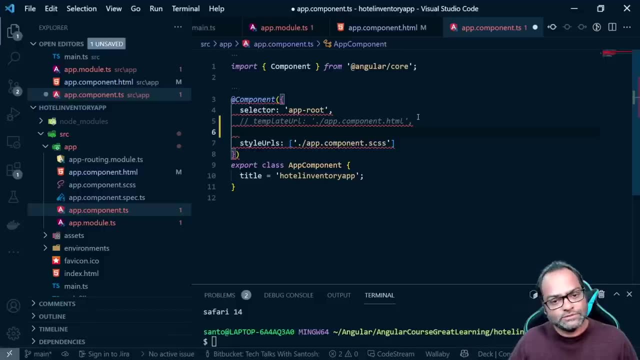 so we have hello world here, but let's see how you can actually make it in line as well. I'll remove this. I'll comment this template url property. we will be using template url. I always prefer having another html file to write our template. in case you want to do it in line, you can use template property. 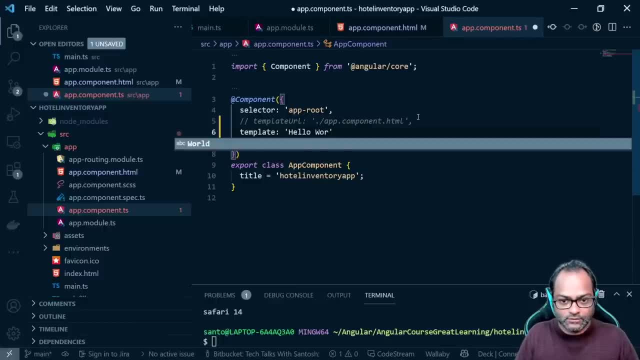 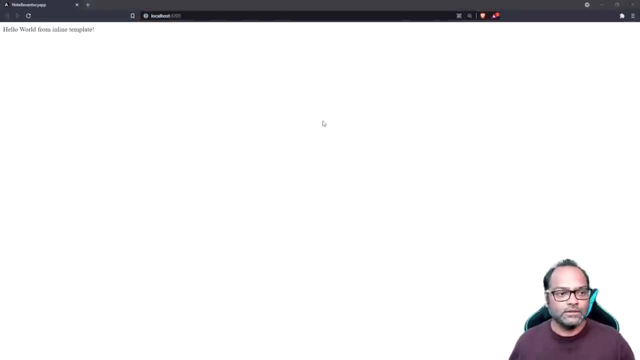 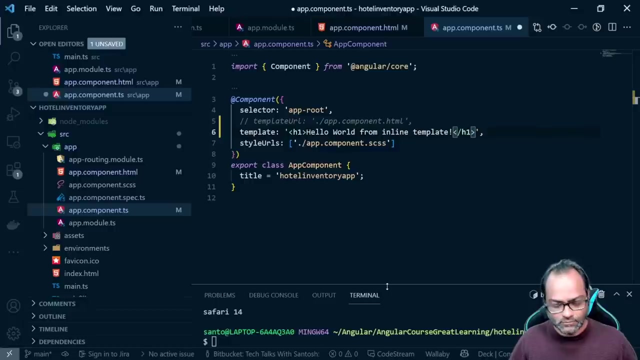 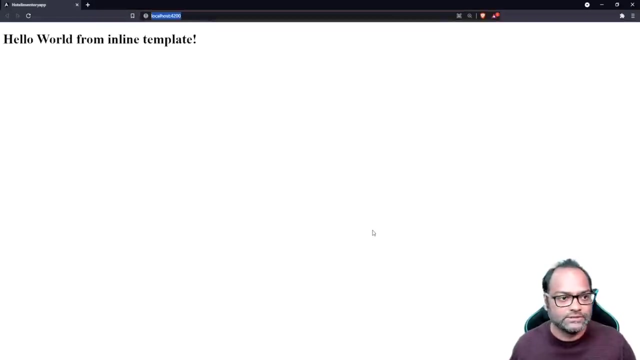 so I can just say: hello world from inline template. right, let's save and you have hello world from inline template, and I can also, of course, add h1. and you can also see I have installed angular inline angular language service. I'll talk about that as well. I was getting an intellisense whenever I write, whenever. 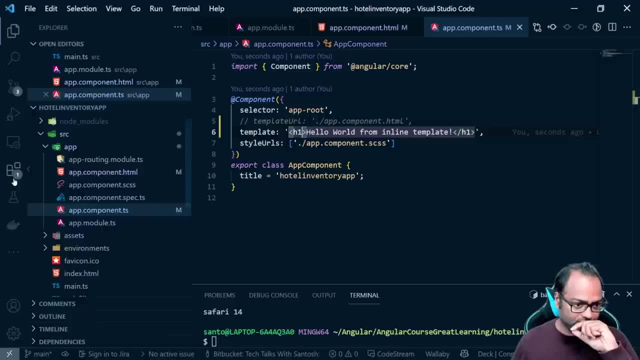 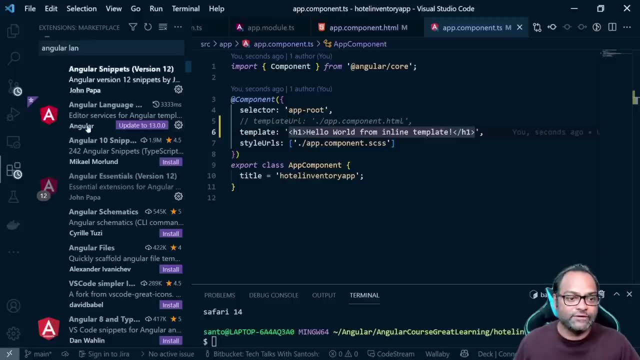 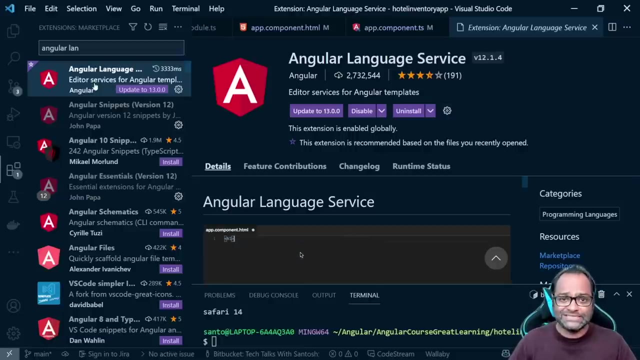 I was writing the inline html tag, so let's, let's, let me tell you you can go to extensions and you can actually go ahead and install angular language service. this is the angular language service. it's created and maintained by angular team itself, so it gives you all the intellisense. 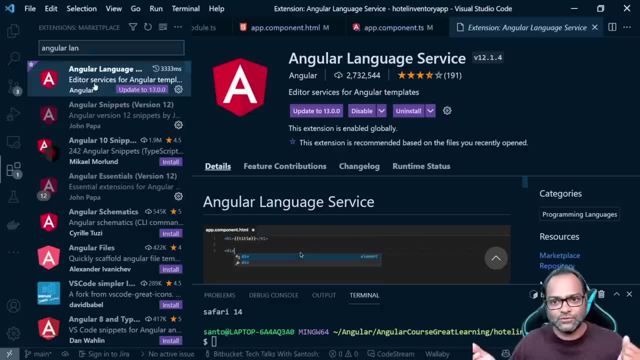 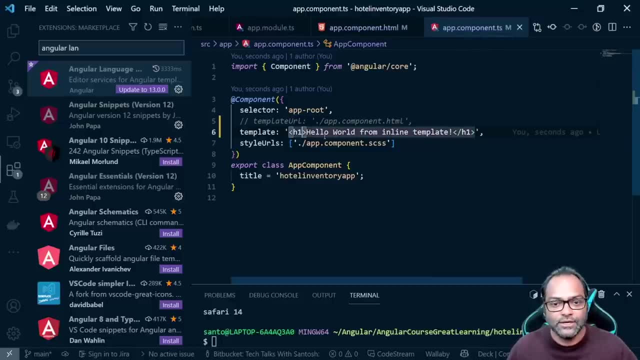 inside your vs code. even it gives you all the errors inside vs code, so you don't have to do it to worry about, like getting those errors while compiling or building your application. most of the errors you will actually get inside your editor, for example. let's try this out, I think. 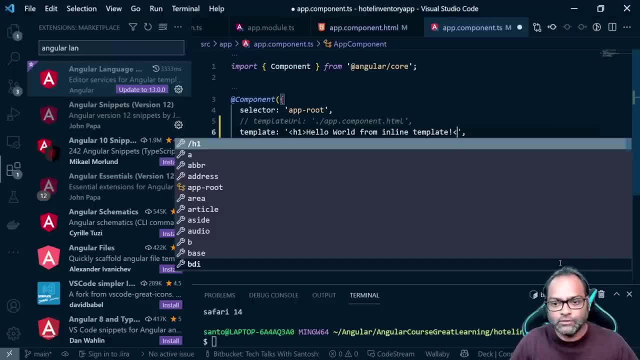 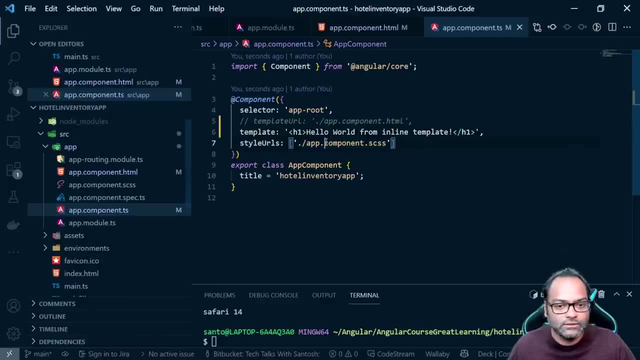 okay, this works. yeah, but here you can see it is giving me option that, okay, there is open h1 tag, so this is inline html template. but what in case you have multi-line estimates sometime you may do not want to actually create a separate file for your template. 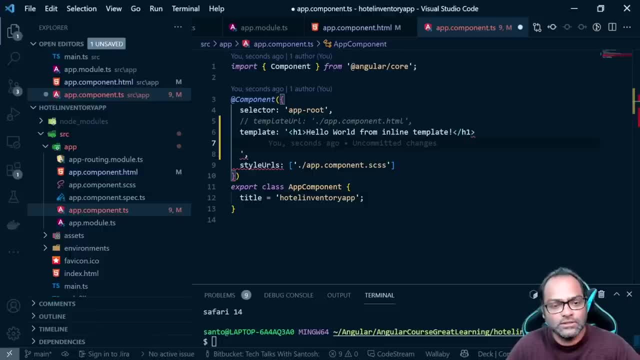 but it's multi-line so you cannot do it in a single line. that's possible as well. so what you have to do is, at a back end of single quotes, you have to use the stick operator. remember, we use this in TypeScript as well. so I can mention the, let us use p-tag and I can use a random type. 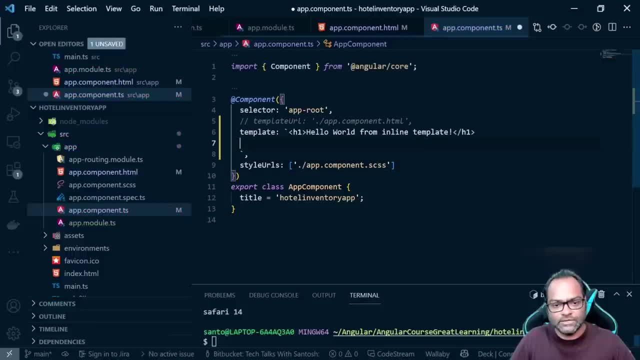 You have to do this any time. you want to type any name, click and you can mask that. so let's do this- example example- here: once you melt this segment, your price isn't fish, it needs to be. it doesn't show, so we need this only take. okay. so I'm only going to close it with product комментでは. 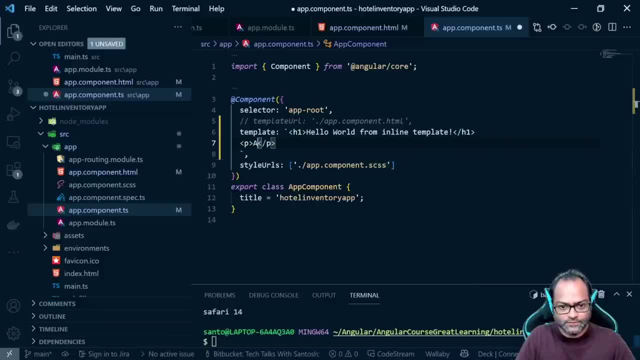 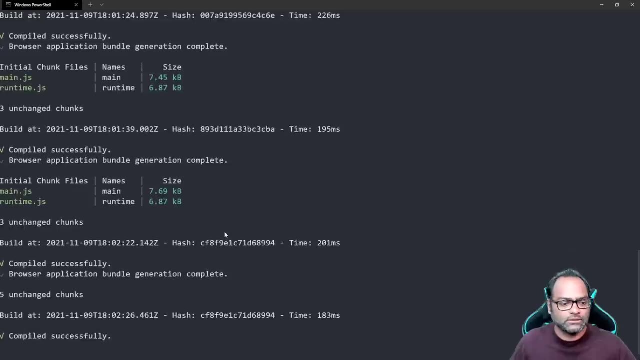 you have email address. people fors, la voi, I have to remove the color. if you don't like text, даже vise, use p tag, and i can say: angular is awesome. and now you have multi-line html right. so just add the this tick operator and then move your html. 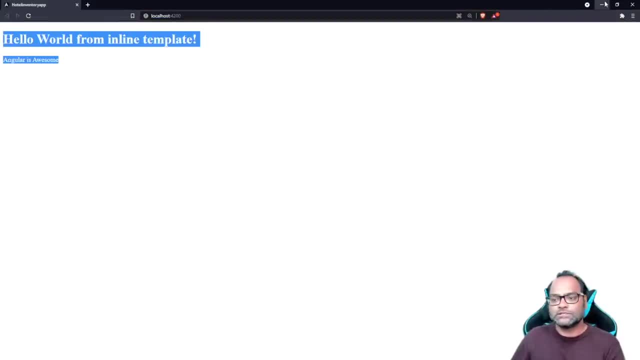 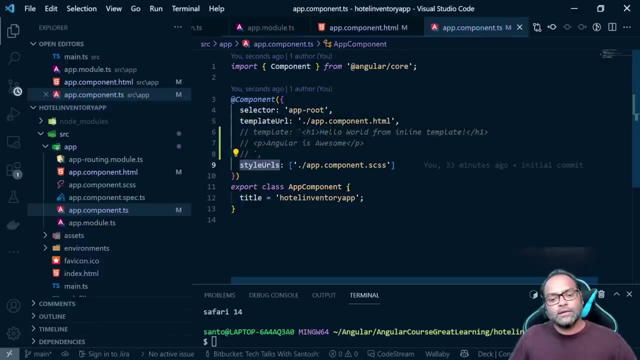 here so you can see. the output is available here. so this is how you can do it in multi-line html as well. i'll just keep this here so you can refer it in future. you have style urls- same, so i either. i can have uh another file to create all the style sheets. 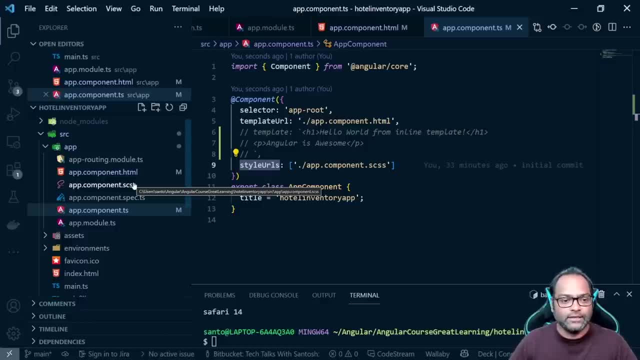 uh, sorry, all the styles related to this component and or i can just have inline styles as well. so it's up to you whatever you prefer. i'm not that good into uh styles. i mean i can probably- yeah, i can- write some css, but i mean i that not that advanced, right. so it's up to you which styles you want to use. 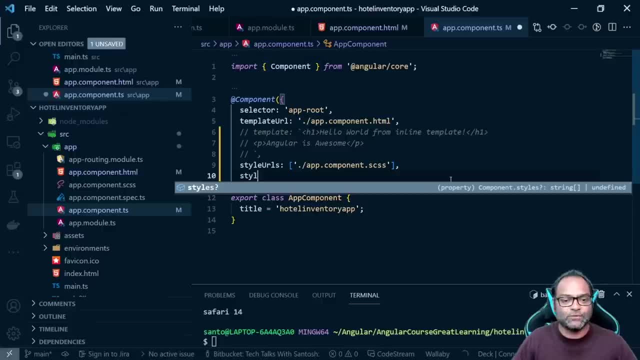 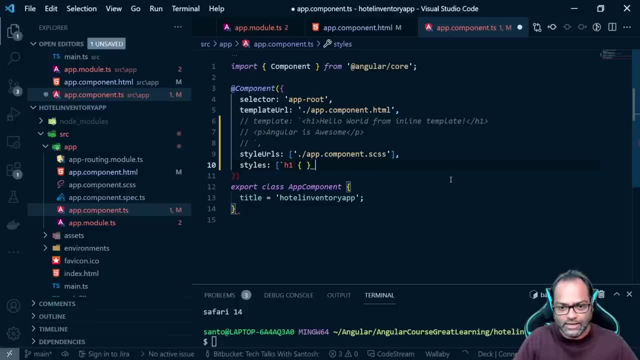 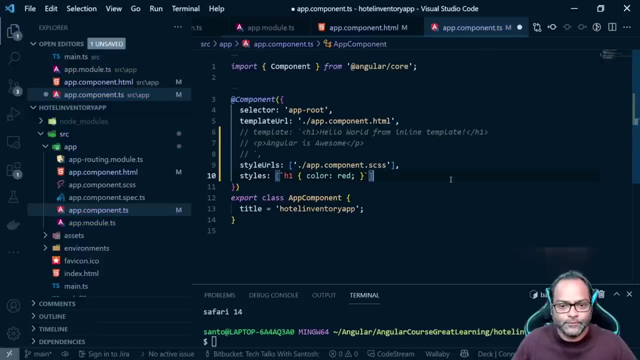 let it be a separate file, or you can also use styles property to give you or to write your inline styles. so i can say: okay, this h1 will have, let's see, i'll comment this one and then we can use inline styles where we are saying: 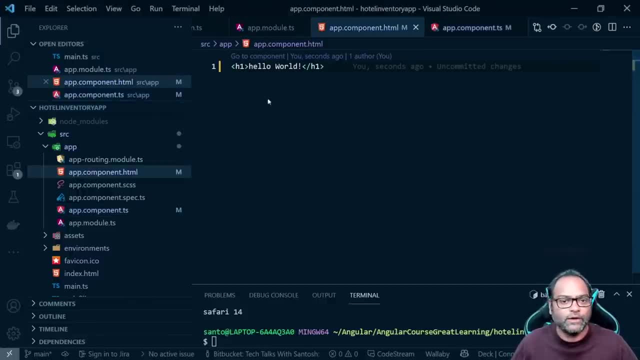 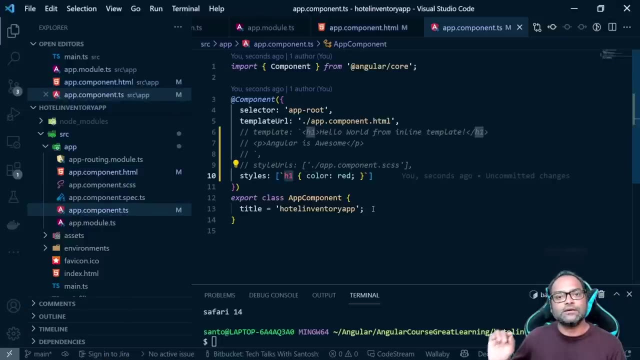 this h1, if we have one. yeah, we do have, and it will have the color red. so this is how you can write it in inline and, as we said, now you can also use inline sas code as well here. earlier it was not supported, so just keep that in mind. with angular 12, it is supported. now i'll just comment. 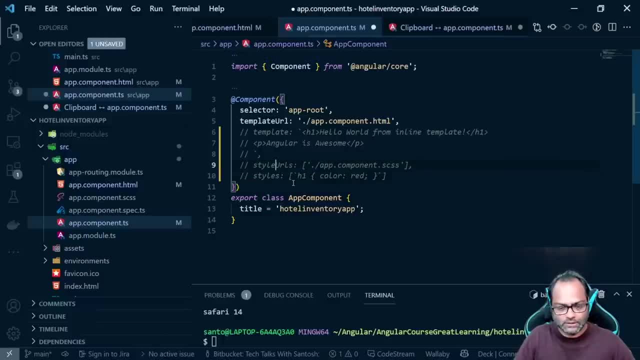 this as well. so now the few fellows i've already submitted, that will be component support. my only component is a terminal dependencies, which is, alas, that's the same thing as a column與 l woman component, and we also discussed about module. so now what we can do is we can create our new. 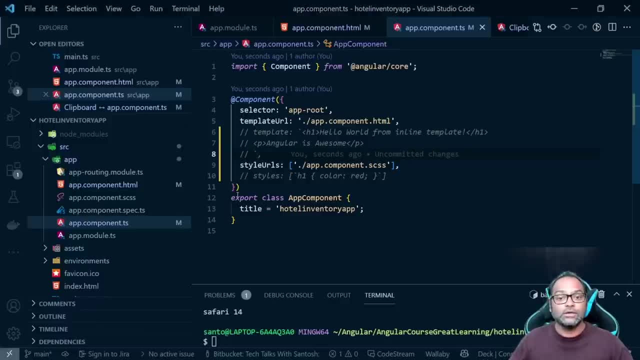 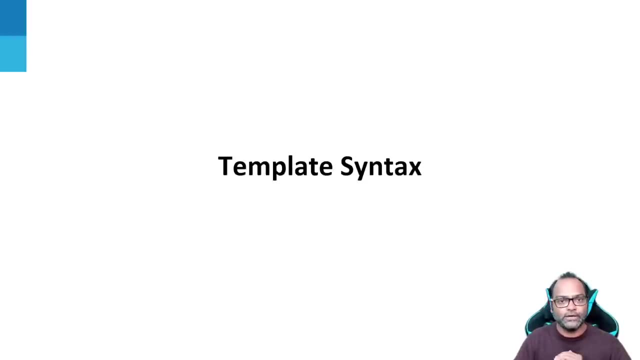 component, and then we will start learning about the next topic or next concept, which is template syntax, because, of course, this is important. whenever you want to start working on a new ui framework you, the first thing which you have to understand is, of course, the language which we 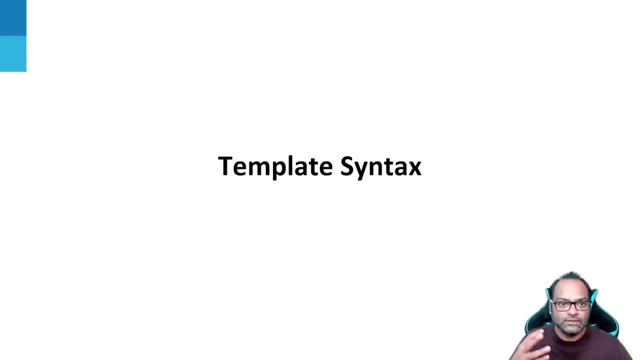 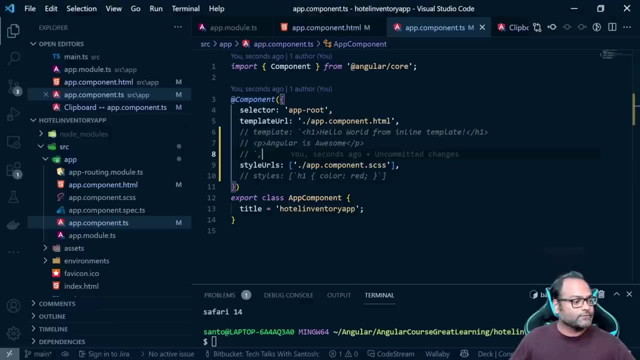 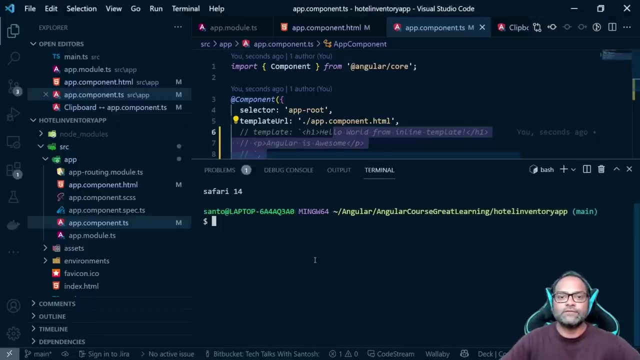 have learned about, which is typescript, and the next thing is the template engine- how to write your templates- and let's go ahead and do that. so, first thing, first, i mean first- what we are going to do is we will be creating a new component and we will be writing our code inside that particular. 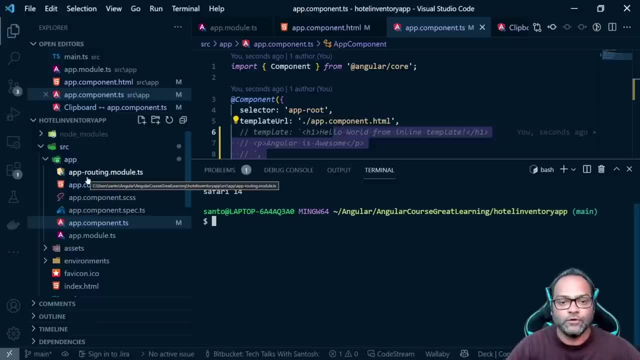 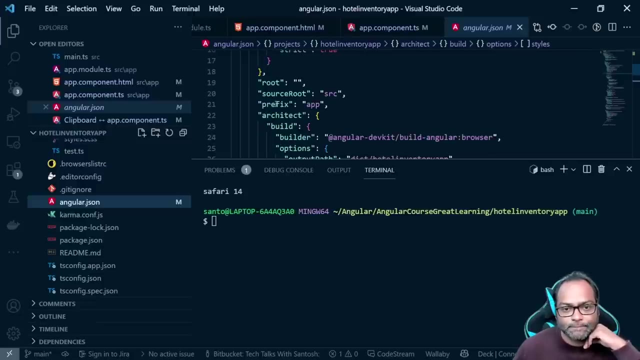 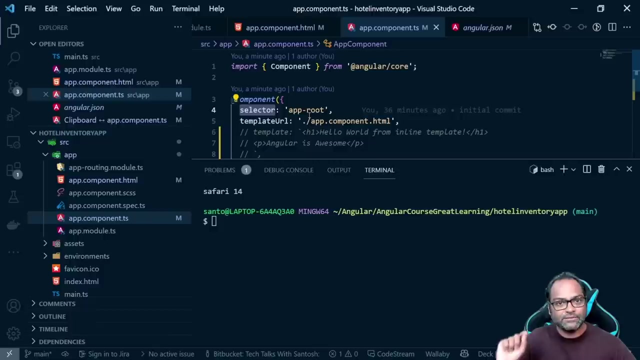 component. okay, before we move on, before we go ahead and create a new component, i want to again talk about the selector property, remember? uh, there was in angularjson. there was a prefix called app. so this prefix is actually used whenever you create a new component in your html tag name. so here, app root is your html tag name and app is a prefix. angular says: 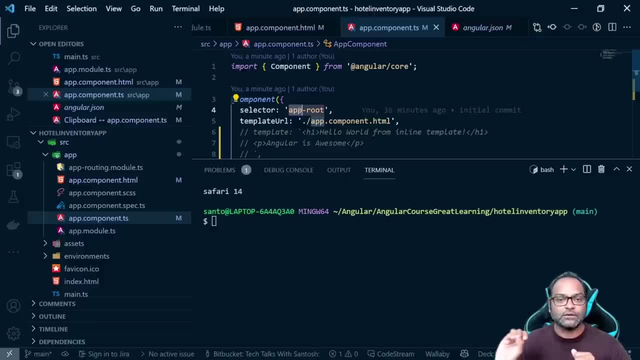 whenever you are creating a new component, have some prefix just to avoid conflict with any other html tag name. so you will be creating a new component and when you create a new component element which may exist. so if i just keep it root, there is possibility that root may be another html. 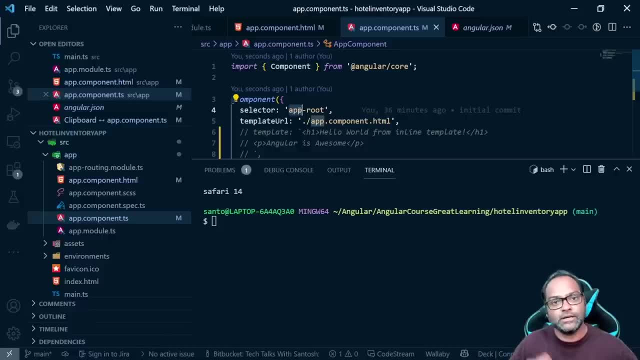 tag defined somewhere. it can be native, it can be created by some other library or it may be created in future inside, let's say, inside html as well. so have some prefix. generally it should be, it should start with: whatever your application is, or let's say: some people also, some, some companies also keep. 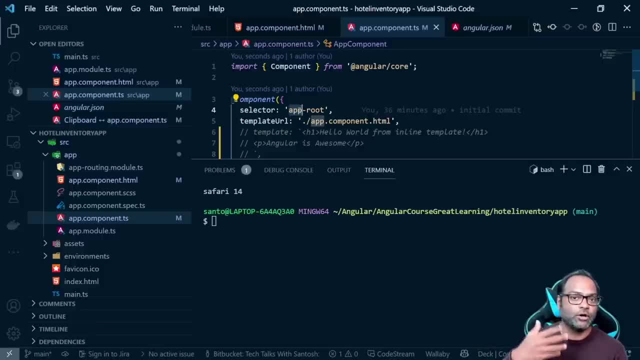 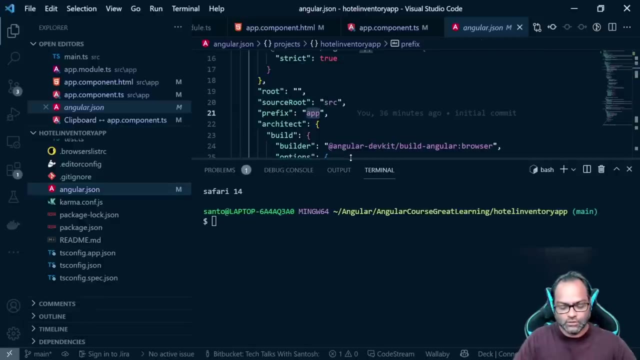 it on based on the company name, right so. or the application name, whatever you prefer. so right now we have app, but we can change it to whatever you want, if we want. so here let's say: i can change it to hotel inventory app- right so, hotel inventory app. so i can say: h i, i know it. 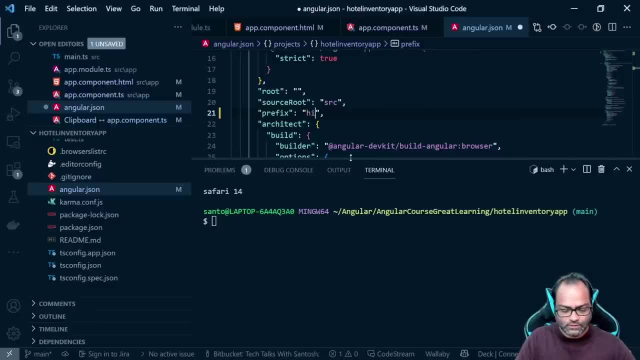 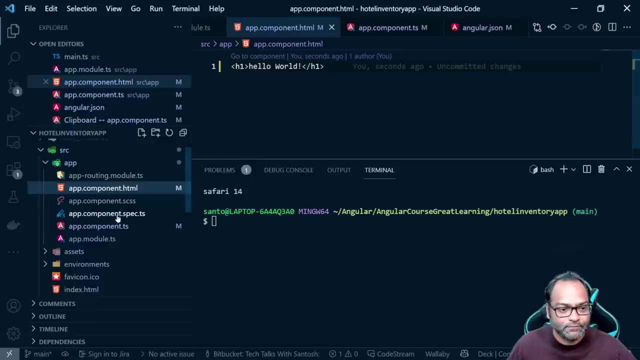 sounds really bad. h, i, n, v. for example, hotel inventory right, so short for hotel inventory. or let's say, if you have some specific hotels right for whom you are creating this particular app, you can keep the select prefix based on that. now, if you change it here, you have to actually go ahead and change it here as well, and once you do, 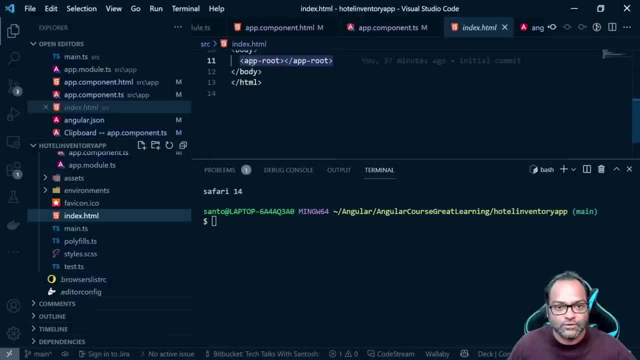 this, you have to go ahead and change it to indexhtml as well. so you have to say, okay, this won't be that Bul carburetor of the summer or whatever. right, and that recall something. now let's say, if you have app route, Ravel is butter, but hotel inventory management. 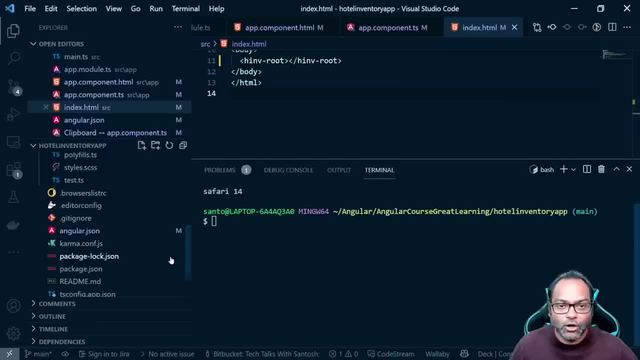 dot hotel inventory rote, right so? or you can also do it while you are creating your app, so you can also do it while you, while you are creating your, so you can say: create ng new your application name: Open files y Evangelical 練 App – Martin. 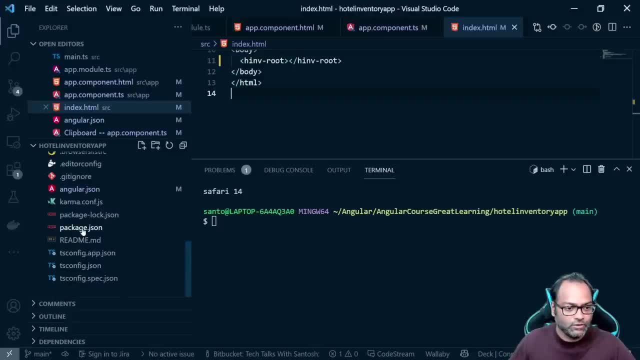 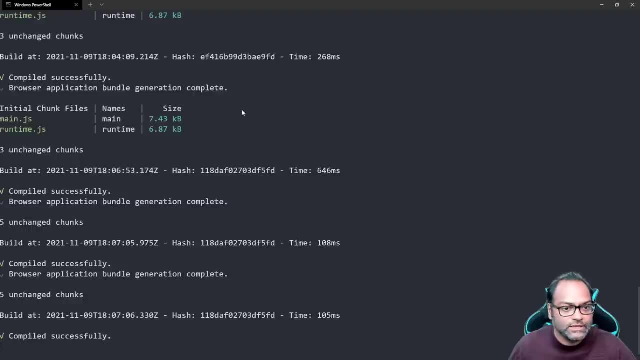 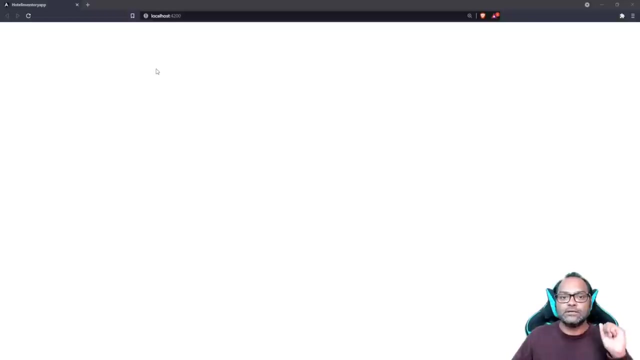 Everything – college October 2019. Anko Ryou Pattern schnell. So let us see if it still works. yeah, as I mentioned, we made changes right now to angularjson and any angularjson related changes are not washed, So we have to stop our server and run it again. 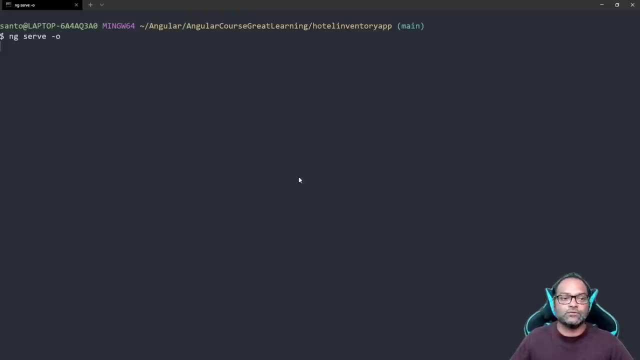 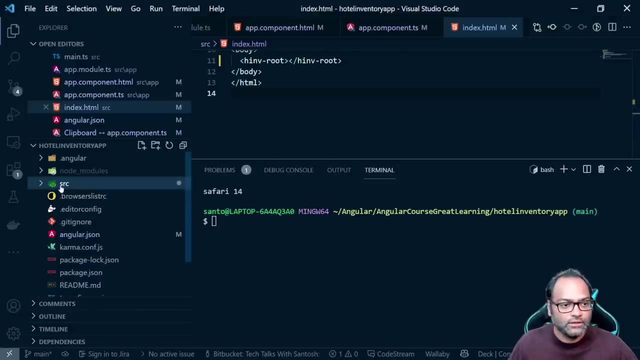 So let us do that here and we will do in the server again, and meanwhile let us go ahead and start preparing or start talking about the new, the next topic, which is template syntax, right. So we will talk about template engine and you have hello world again. 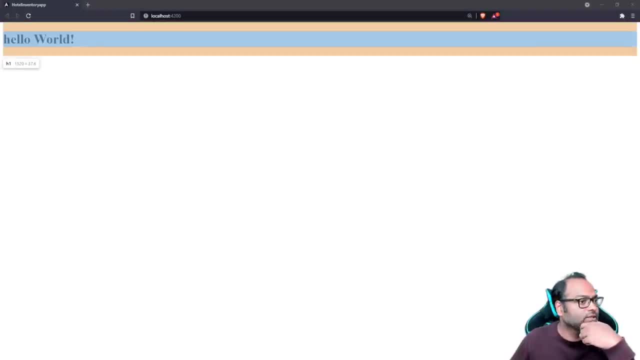 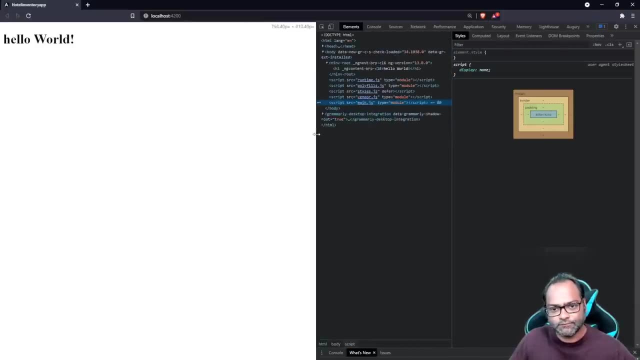 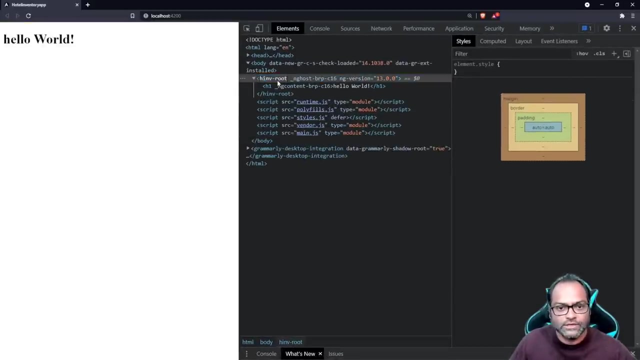 But if you see hello world, I mean, just let me show you one more thing here I can go to inspect and here you will notice, This is your estimate html tag h, i n, v, root right, and then you have h1 tag available here. so this is the html tag you. 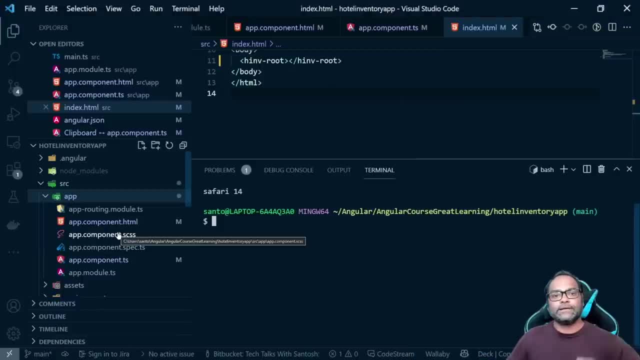 created right now, yep, time to create our own component. so here, uh, what we will be doing is we will be creating, um, we will be creating a hotel inventory management app. so let's create some views around that, right. so first, what is important if a hotel wants to manage its inventory, what is? 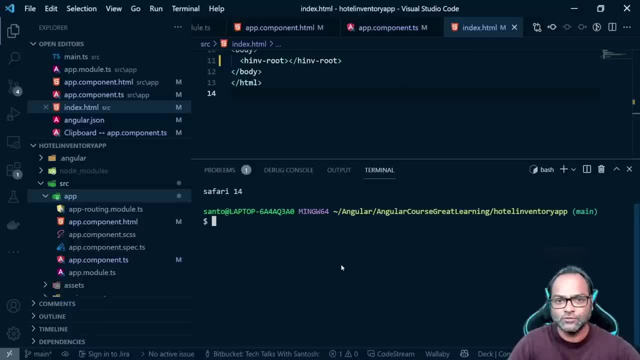 the most important inventory: rooms, right, so rooms is the most important inventory they have. so what we will do is we will create a component. so how you can create a component is you can say ng, g, which is short for generate, so you can also write generate if you want to. 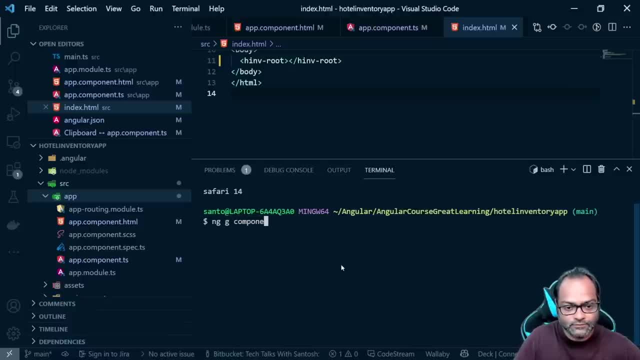 we'll be using shortcut and then you have component, which is also there is a shortcut to write. we can write c and then your component name or your view name, whatever you want to give it. so let's say: uh, i want to now create a component called rooms, so which can have information about. 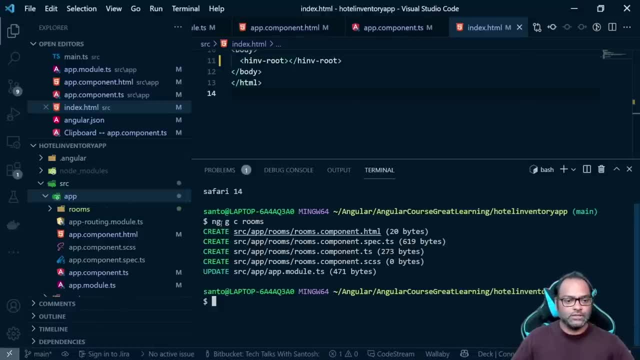 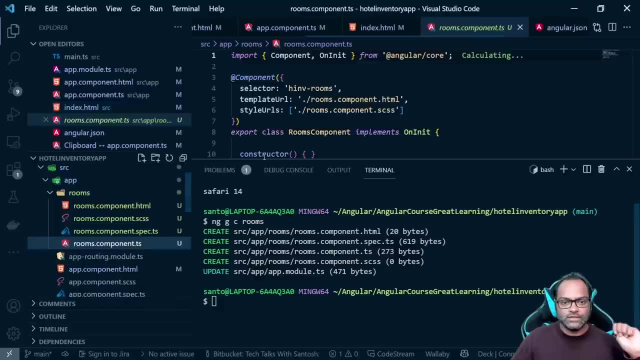 all the rooms the hotel has right now and whenever. you do that, as we mentioned, this will create four files. you have html, css, pegts, and then your ts file is where you will be writing your code, html file where you will be writing your views to get. 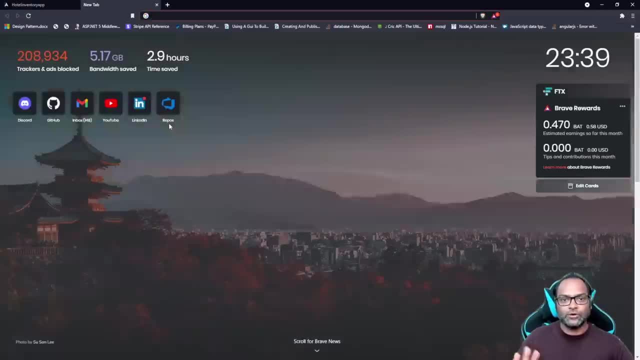 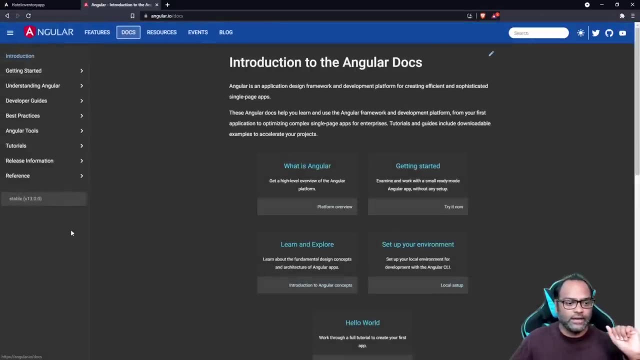 the list of all uh commands. you don't have to remember those. remember just just keep that in your mind. you don't have to remember all the commands, all the options. you can just go to docs and at the end of the docs you have the cli command reference and you can read all the commands in. 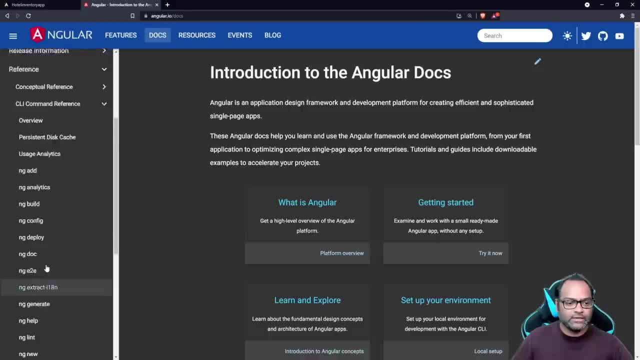 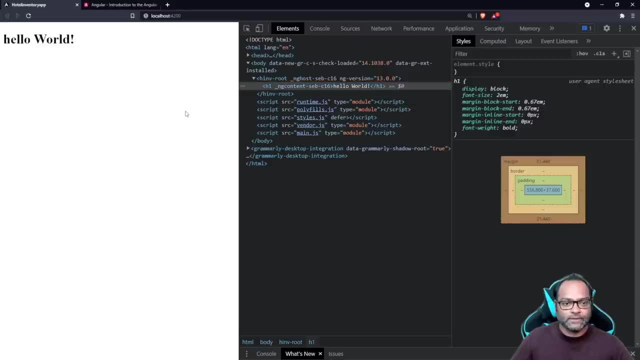 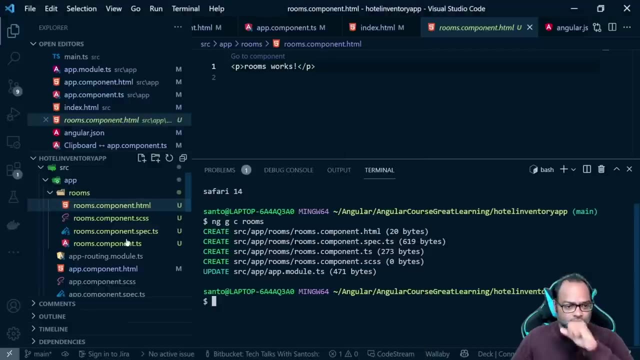 case there are some changes in future there that will be updated. in case you get a new command in future, that will be added here as well. so you have all the information related to cli commands and this is our application. so let's close this. so now we have created our first component, let's try to right now, just uh. 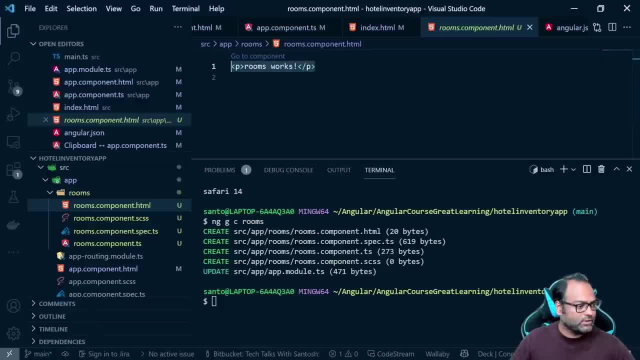 see what is here. it says room works. let's go back to our application on. sorry, let's go back to the browser and see what is available here. so we just have hello bird. so in case i want to render this rooms component or any information related to rooms component right now, i have to add this html tag here because 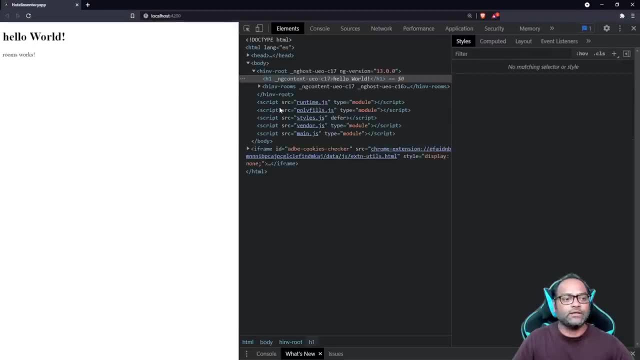 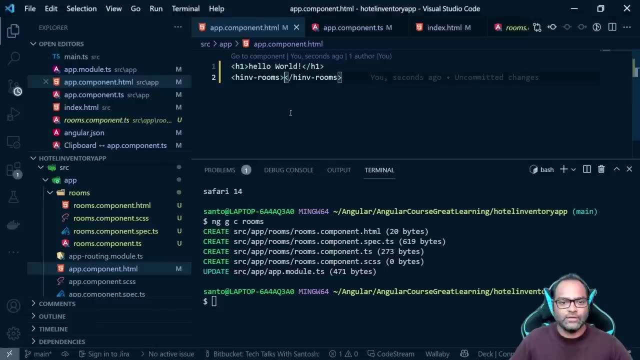 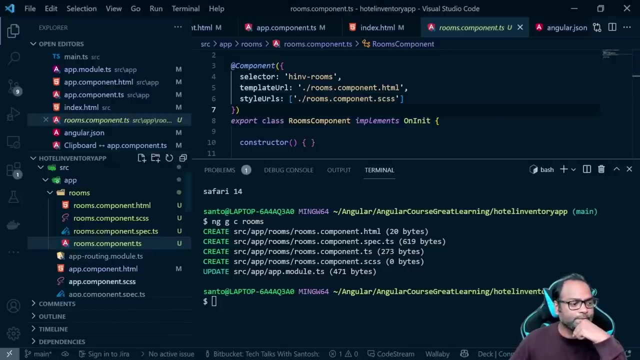 this is our entry component and you will see, okay, it says rooms work. it means the new component which we have created is getting rendered perfectly fine, you don't have to do anything. let's go ahead and add some information. so let's talk about templates. first question: why do i need to do this? 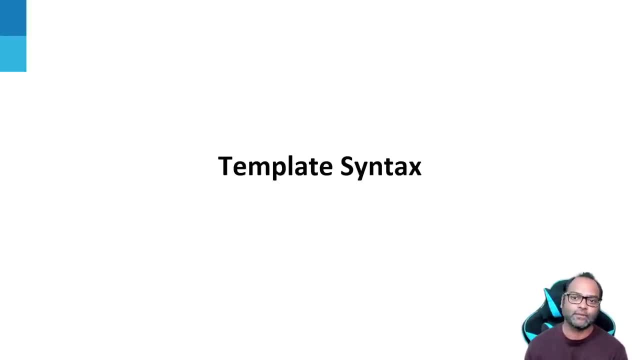 let's talk about templates. first question: why you create front-end application. okay, if you are wondering, you get paid for it. yes, you, that's. that's the different uh answer. but what else? right? so we create front ends because we want to display some information to the end user. that's the whole purpose. i mean, of course, i can create apis and 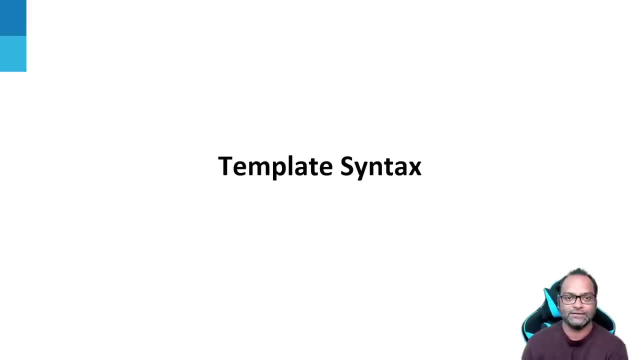 i can ask my users to just hit those api and get information right. that that's- uh, that's developers, that's that information is relevant to developers. but for end users, the information which is available on some some front-end application, that's what matters. so you get paid for that and it means 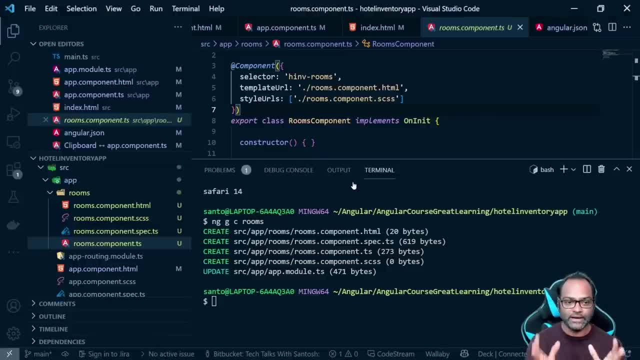 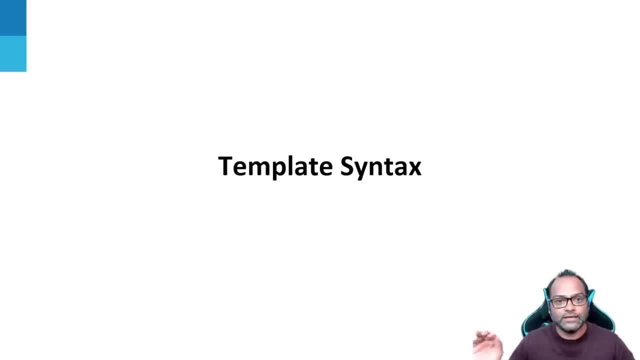 whatever code we have to write, we have to eventually go ahead and bind that data to our html. our view, that's where it will be available. so let's start. let's see how you can actually do that in angular. every uh language, every library, has their different syntax to. 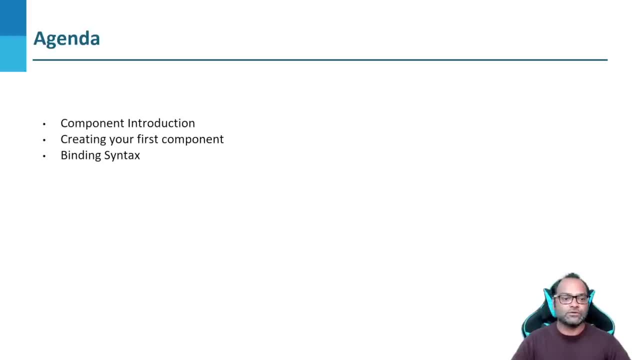 work with templates, so how you will do it in angular. so here we have already, uh, discussed about component introduction. we have also already discussed about how great you you can create a first component, so we'll just skip here and then we'll come back, come to just binding syntax. so let's see, so how you can bind that information to your front end. 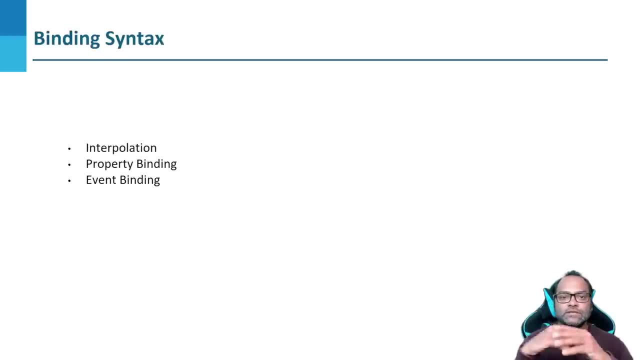 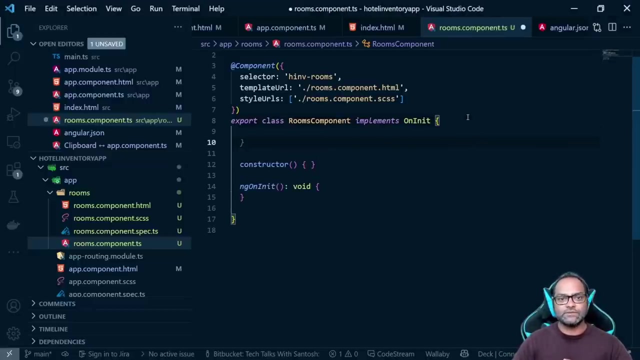 let's close this. so there are three ways, uh, to bind your information, which is available in your ts file, to your html. so you have interpolation. you have property binding, you have event binding. so let's see first interval, interpolation. you can use interpolation syntax with any basic data. 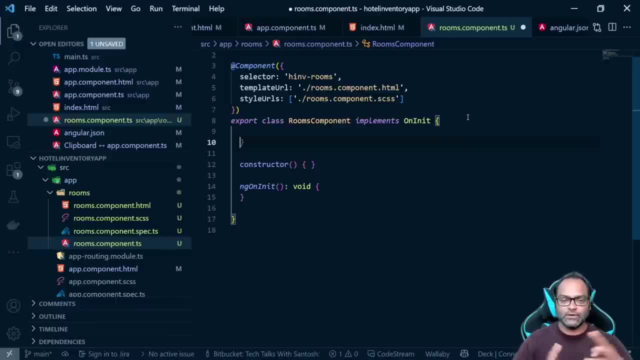 types, for example, if you have date, if you have string, you have number, uh, those information can be binded using interpolation. even, uh, you can work with objects into using interpolation. so, uh, let's see, what we will do is we will create, um, let's say, hotel link. so this is my first property. 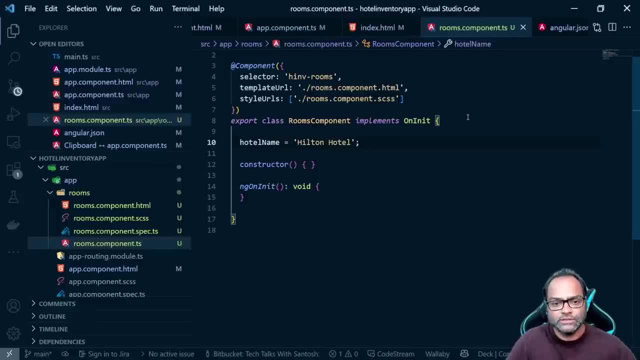 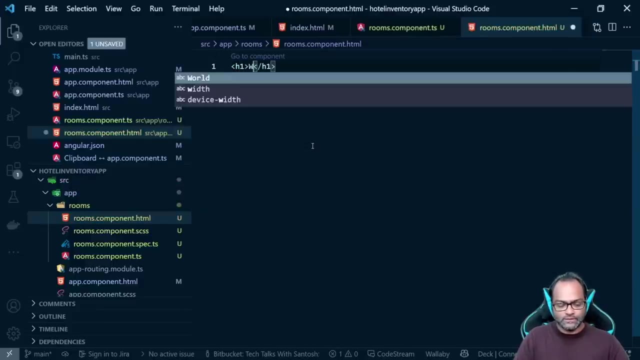 and i'll just print hilton hotel, right? so this is the hotel name for, like, let's say, this hotel name you want to display on our view right now using interpolation syntax, so you can just go to html. i will put an h1 tag here, right, and i'll say welcome. 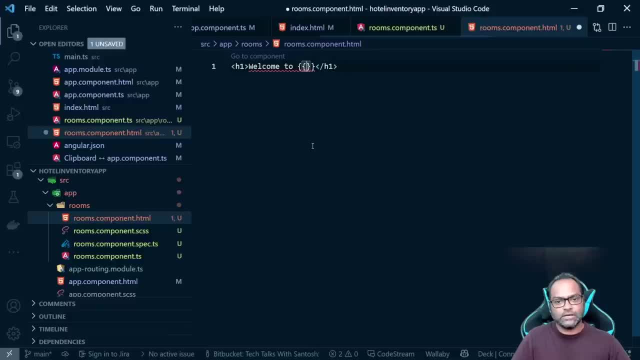 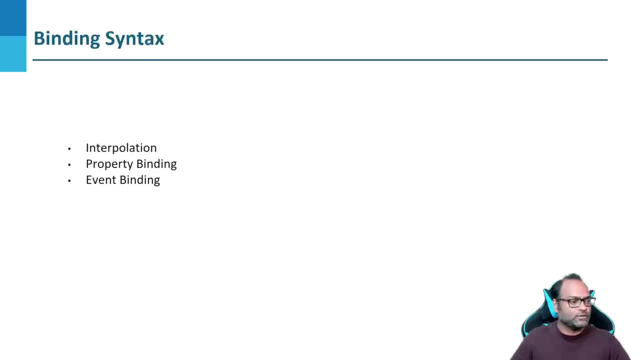 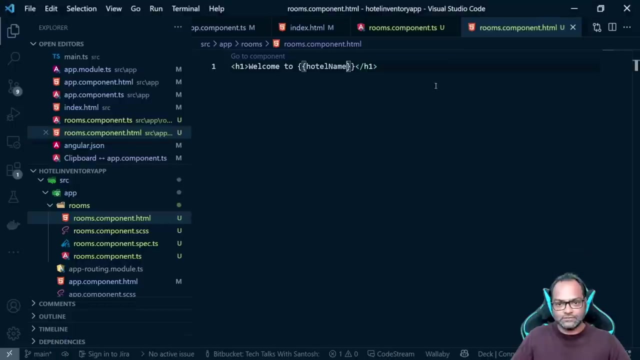 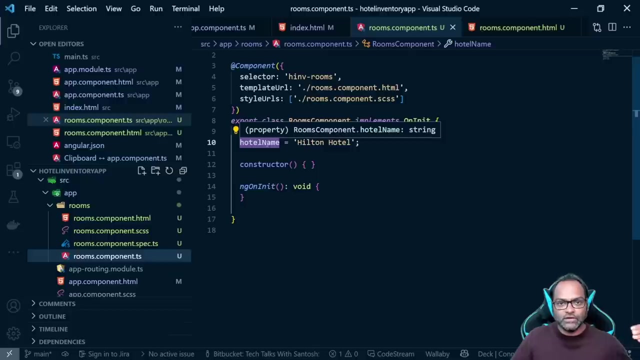 welcome to. and you can put double curly brackets and put your variable name. so hotel name is my variable name, right and just save. let's go back to the browser and it says welcome to hilton hotel. so this is how your interpolation syntax works. so this is string of a variable of type string. you remember we said inference, so it is able to infer. 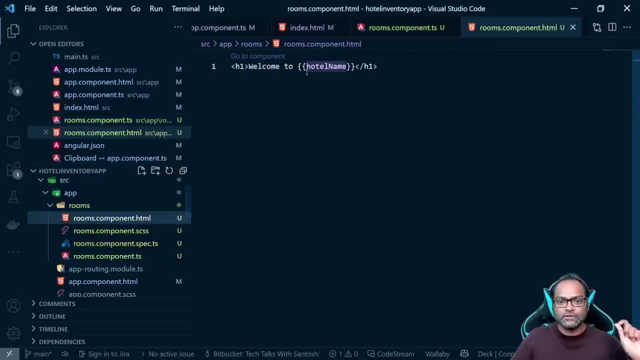 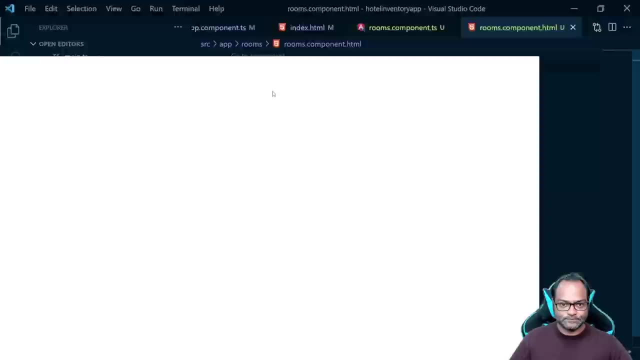 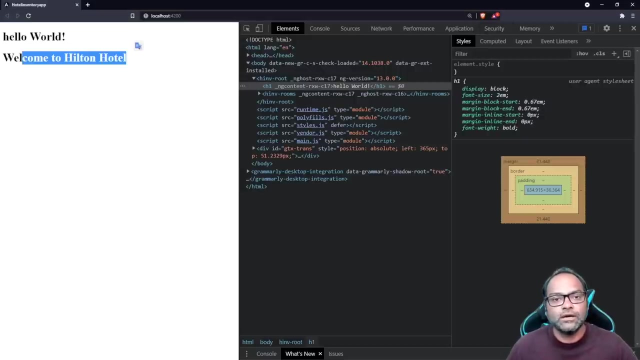 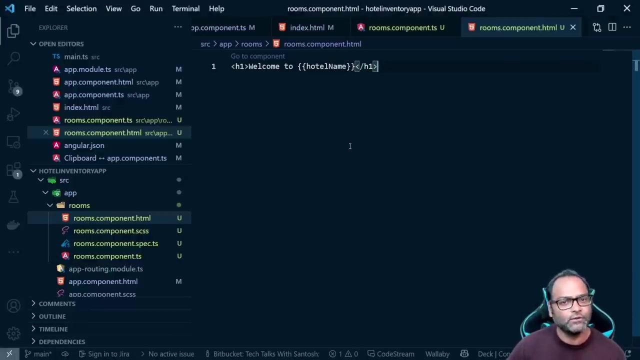 that. okay, this property should be string, and then we are displaying it using the interpolation syntax. angular allows you to also use. so let's talk about the second way, which is property binding. so angular allows you to actually use native html attribute properties for binding as well. so what i mean by that? so 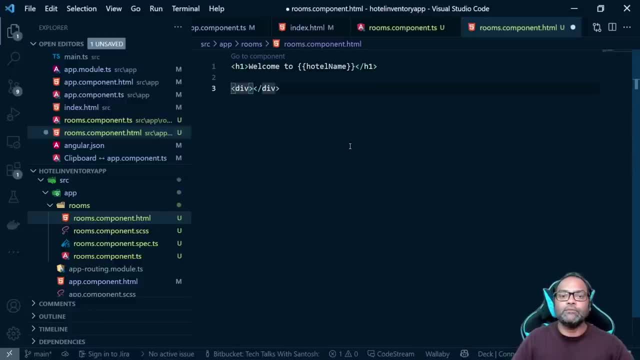 actually i can have a div and i can bind a value directly to this, this div to any valid property of this particular div. so remember, do you remember any uh valid property of div? so in case uh you don't, it's absolutely fine, you can just go to uh mozilla docs, right, msdn, and read. 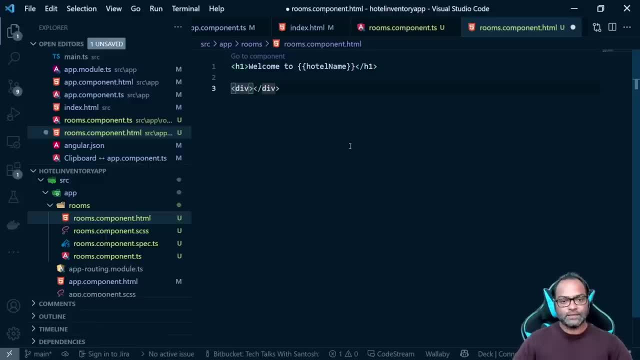 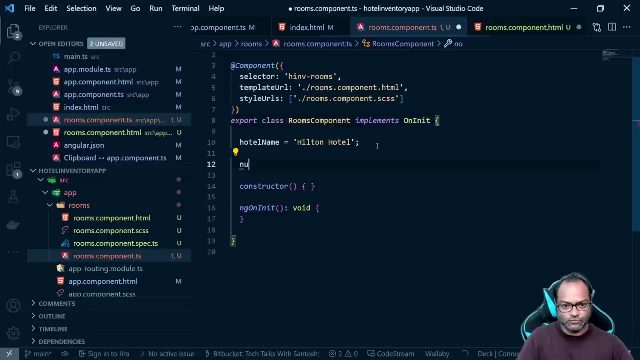 about all the html tags and basic javascript. so i'll use one property, which is known as in a text. so there is a property called inner text equals to. i'll say: here i'll create another property. i'll say: this is number of rooms. so let's say we have 10 rooms available in this hotel. 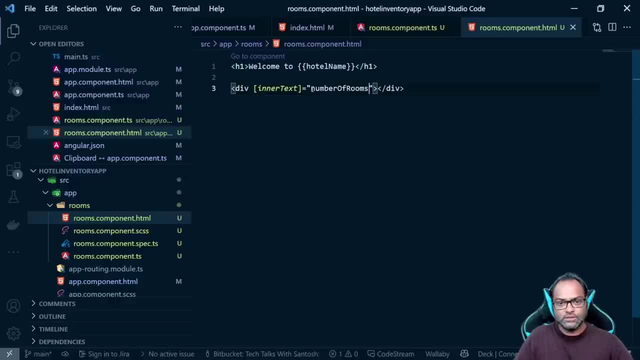 and then i can just use number of forms here. so what is the difference? so generally, uh, you use this in a text property, something like this: this is: this is a javascript code. so generally we do document dot, get element by id, and then you get an element by id and then you apply in a text this: 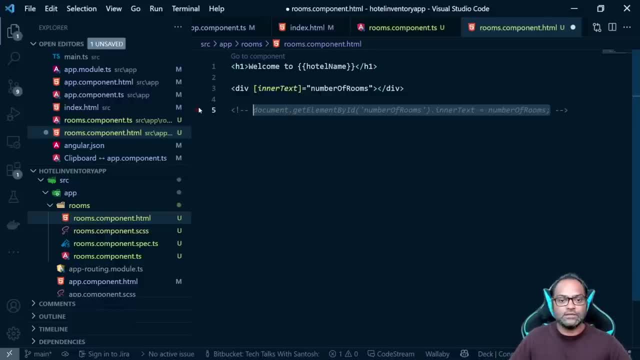 is normal javascript. this is how you do it in javascript, but in angular you can actually just avoid all this code and just directly do it here, and then you get the element by id and then you do do it here, So you have inner text. Remember this box, that's the extra layer of syntactical sugar. 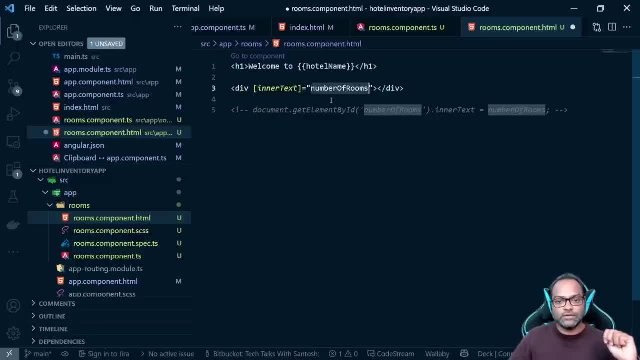 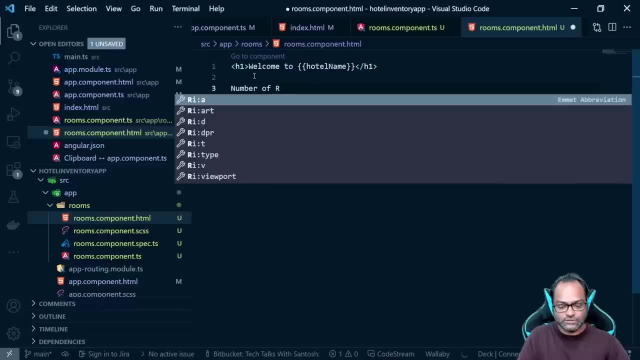 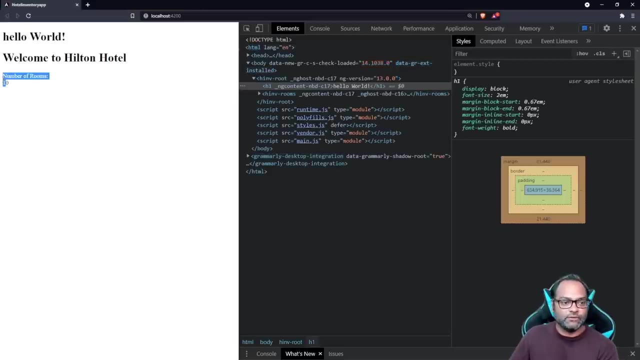 which we are adding, which Angular is adding, And then you are just saying, okay, this variable name should be bound to this inner text property And I can say, okay, this is a number of rooms And you will see number of rooms available then. So this is property binding, Remember. 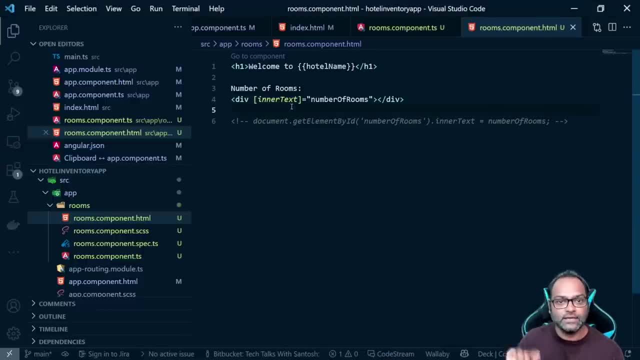 you can only use it with any valid HTML property of any valid HTML tag. If I try to use inner text, I'm getting inline error. Remember I said Angular language service can give you that. That's it. If I save this, you will also get this information everywhere, So you are getting this. 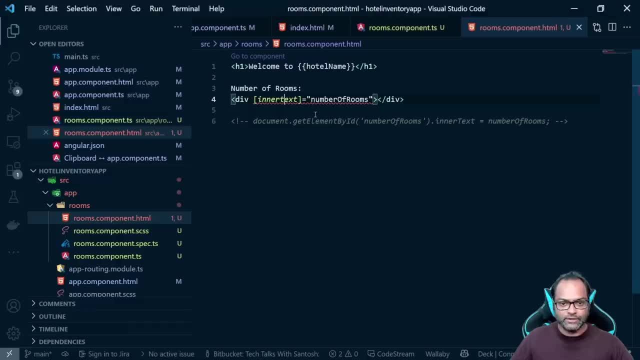 here. You will be getting it in your command line And as soon as you fix this and say, okay, this is the property, it will be gone from here. It will be gone from your view. So it's back and that's it. 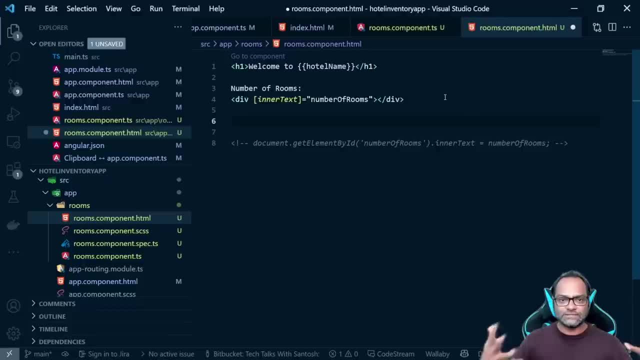 Now, once you create front end, of course you need to display information, but you need to do one more thing as well. You may need to actually collect information. So how to collect information? So, of course, you may want your user to interact with your application. It means 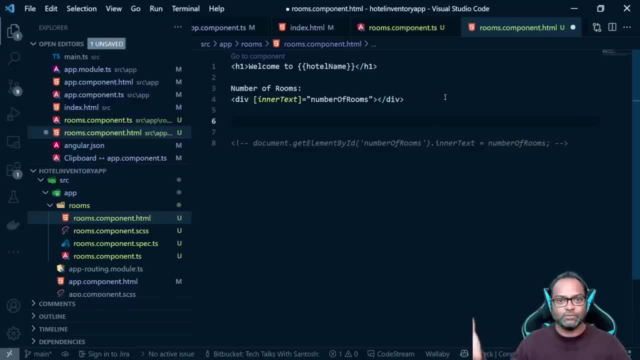 you may want your user to raise the events. I mean, probably save some information or probably, in some cases, retrieve some information based on some filters. So you need those right. So you need a way to actually raise the events as well. 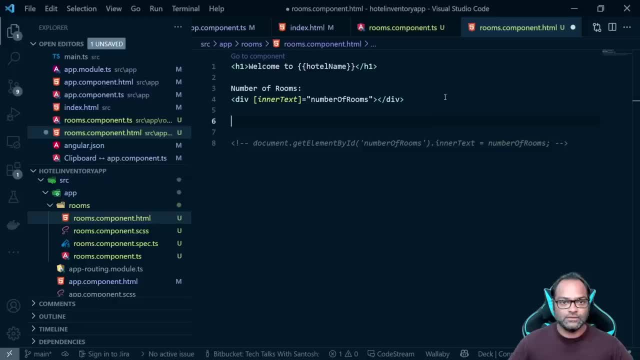 So the third way is something which is known as event binding. So let's talk about event binding now. In plain JavaScript, we just do something like this: So let's create a button and we use click equals to a function name. So here you probably. 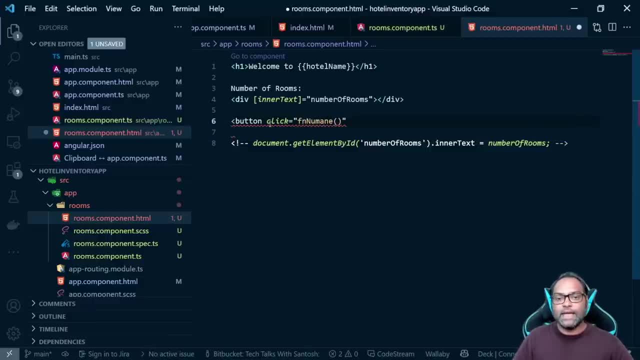 will be using a function name in JavaScript. In Angular you will do some just a little bit extra. So here, sorry, In JavaScript you say on click, so you'll be doing something like on click equals to a function name In Angular. as I said, every programming languages or every framework has their 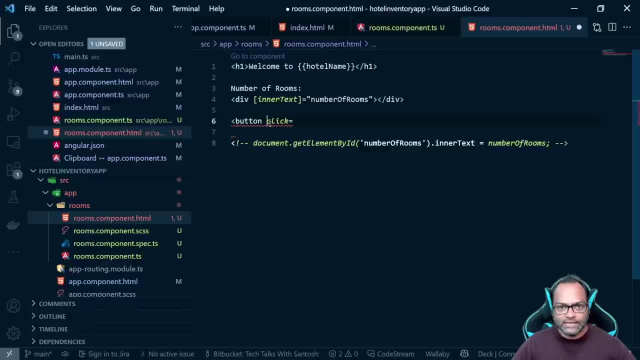 own different template syntax or template engine In Angular. you have to just put it in this banana syntax. so this, this is known as banana syntax and this is known as box syntax. so you'll put any event, just remove on, put a banana syntax and that's your angular event now on. click equals to. 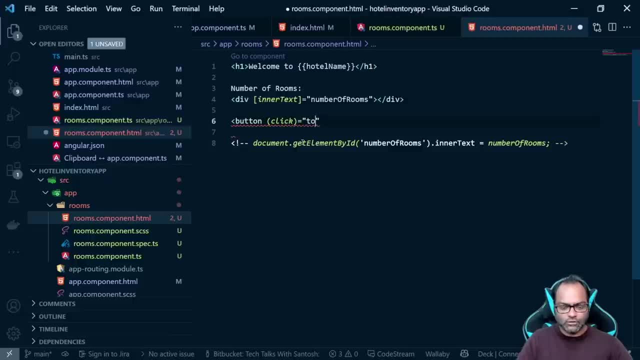 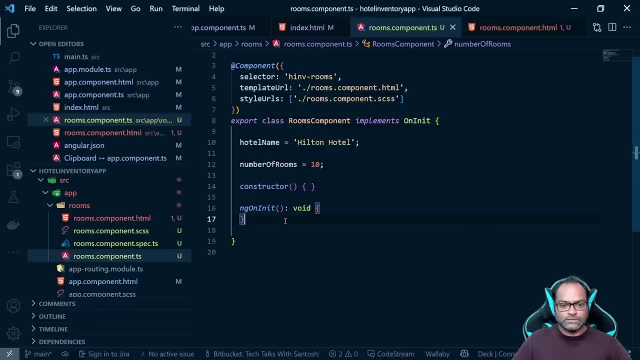 i can create a function. so i'll create a function called toggle and i'll say: this is toggle. so right now we are getting an error because this toggle function does not exist. let's go ahead and implement it. let's go to ds and write a toggle function. 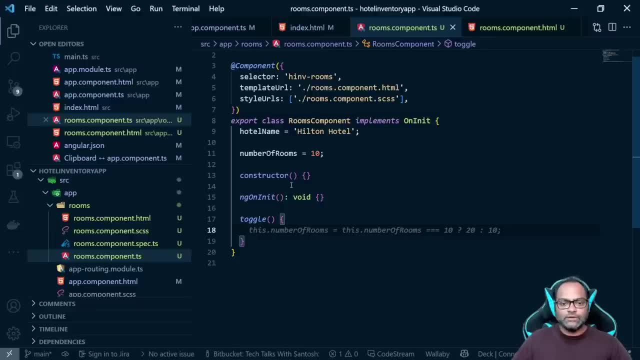 and what this toggle function will do is, let's say, it will hide, show, hide the rooms. so i'll create another property- hide rooms- which is equals to false. and whenever we click on toggle, i'll say this dot hide rooms is equals to not this dot hide rooms, right? so we want to toggle the value and here i'll create a div, here. 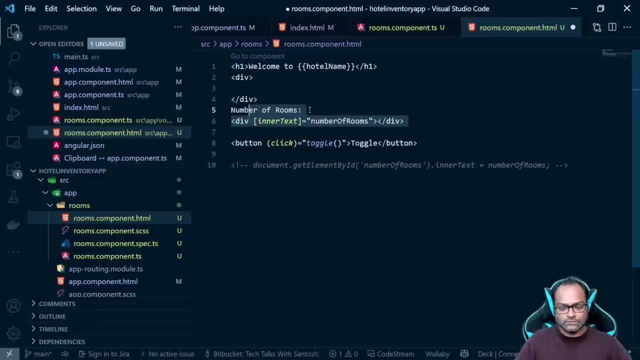 and i'll move this information here, and then we will be using a property binding syntax. so, uh, hidden is a property which i think all available on almost all the estimated tags which exist. so hidden equals to hide rooms. it's a boolean property, right, so true, or 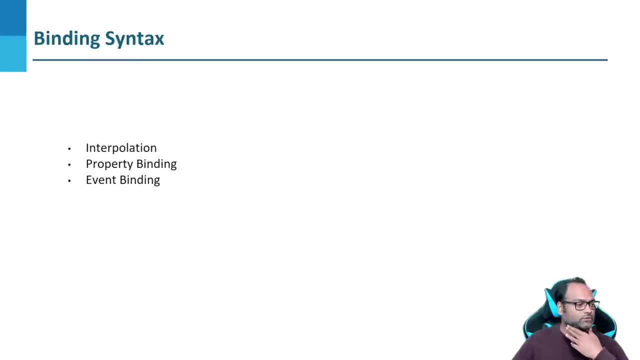 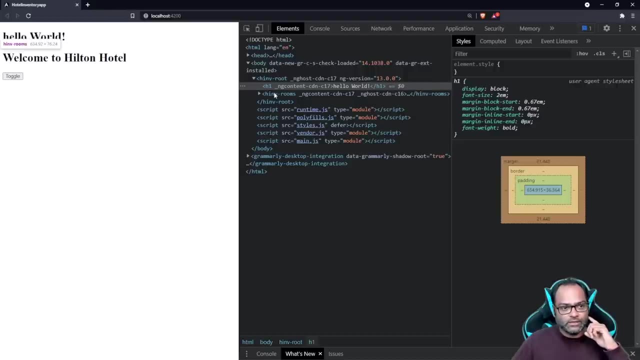 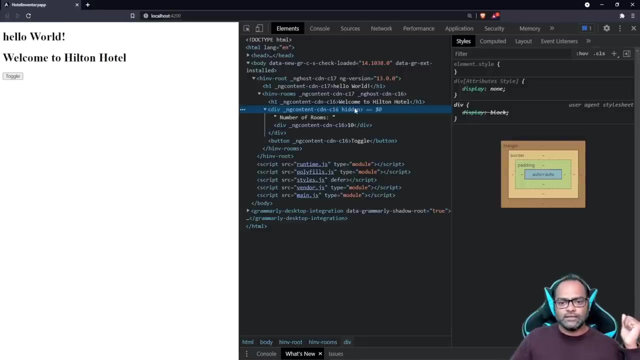 false also true, let's see. so let's go back. so right now we have number of rooms. click on toggle and they are gone. so remember. but uh, this, this div still exists here, right, because hidden is a property and i can just remove it and then display this information again. so, toggle, uh what? 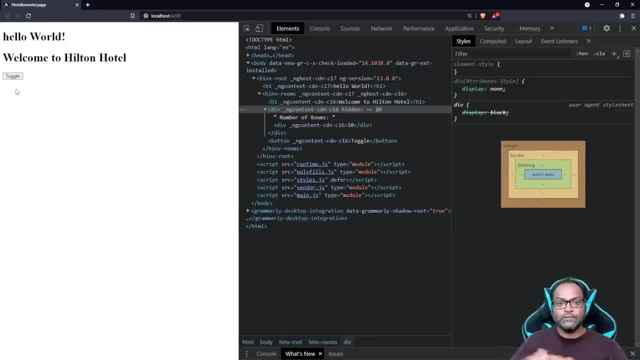 we are doing is we are raising an event which is going and going ahead and updating a property, and then our view is updated accordingly. i'll show you one more thing: how you can actually debug your application, because that will be beneficial for for upcoming videos and, in case you get into some issues, you will be able to. 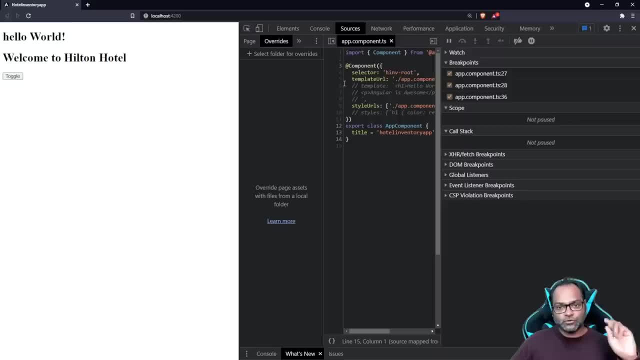 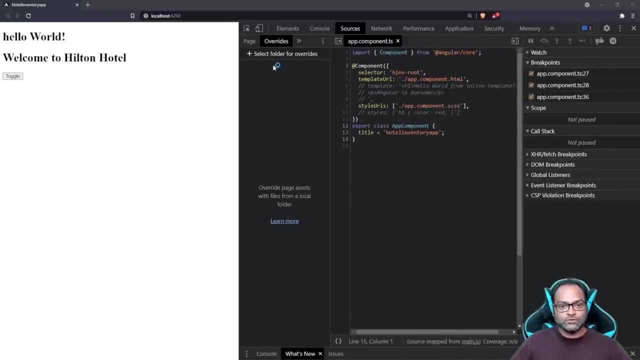 figure those as well. so here in sources panel you will be able to see all the components, all the files which you have written. this is your code, right? so i can just go to, not here. so go to pages and you will be able to see all the files in dot folder. so you, you will be able. 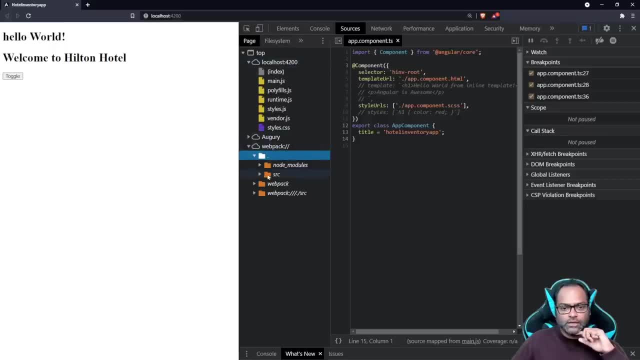 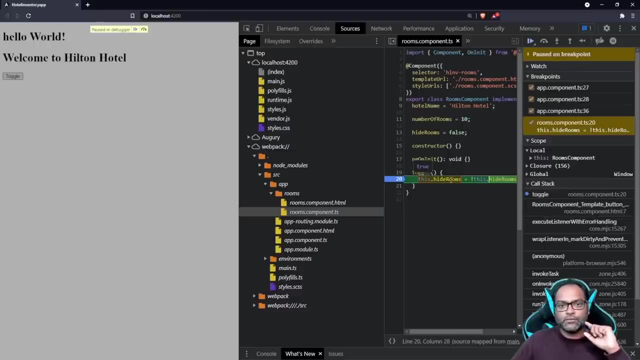 to see localhost 400 and then you will be able to see webpack, and then dot folder is where your code exists. so app, and then you have your rooms and you have your dot ts file. let's add a break point here. click on toggle and you have your breakpoint available. right, so your debugger. 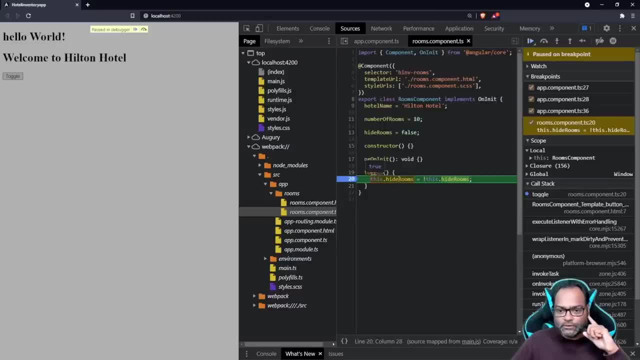 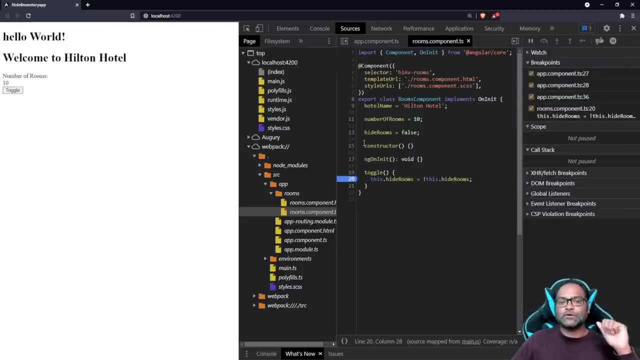 available here, so you can see: okay, uh, right now the hide rooms property is true and we are updating it true, true to false, and now it is available here. so this is how you can actually add breakpoints, find files. you can also use a shortcut so you can. 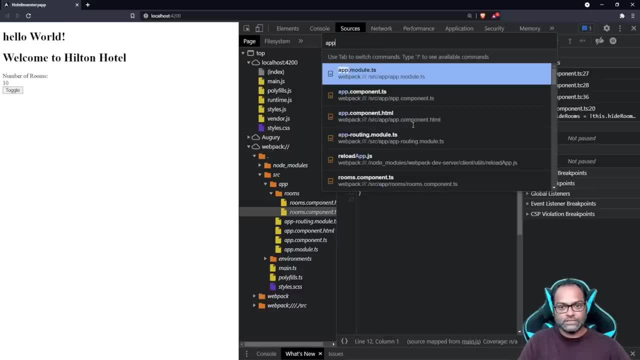 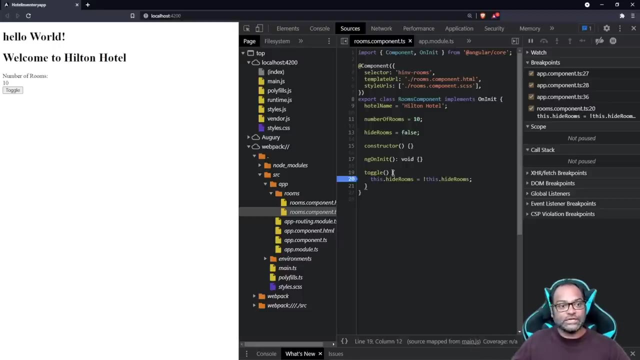 press ctrl p and open any file. so you can just type app, dot. so let's say, i want to open app module, so if you can here, do that here. or let's say rooms, right, so i can just say rooms, dot, componentts and that's it, so you can also search, in case you have a lot of files, of course you. 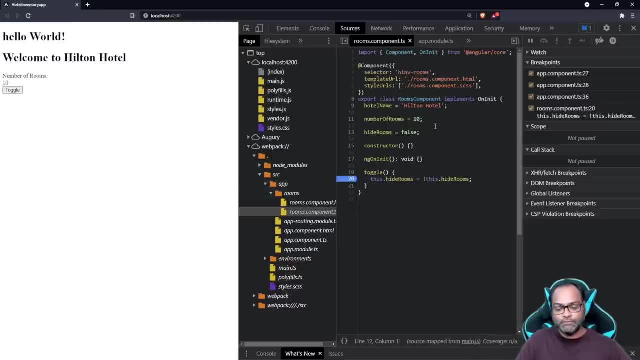 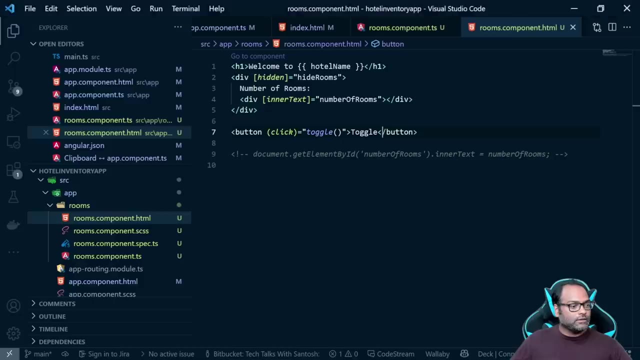 won't be wasting your time going through it. you can just open the sources panel, press ctrl p. this is on windows, uh, in i'm sure. probably this will be the same across all the uh different os for chrome. so ctrl p and then just type the file name. the same command, ctrl p, works for your. 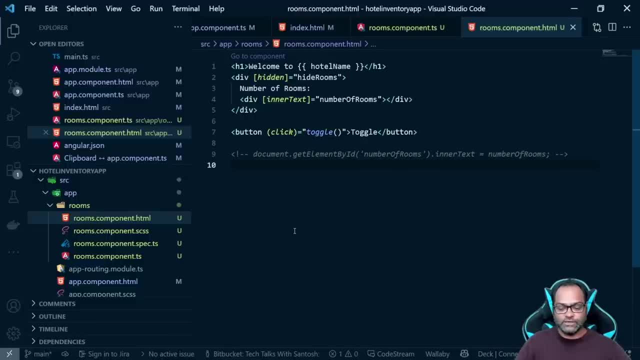 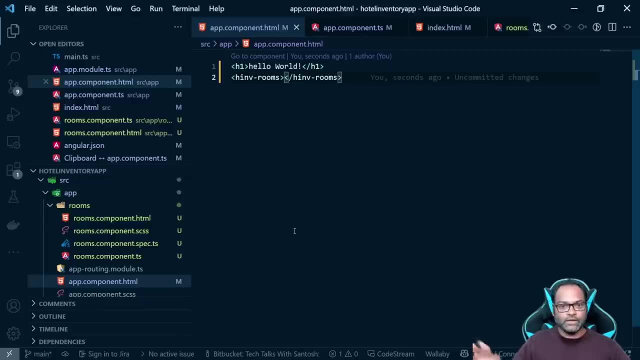 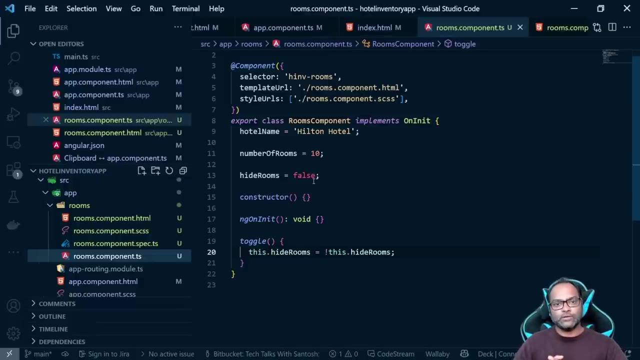 vs code as well. so let's say, if you have thousands of files, how you will search for a file? you can press ctrl p, start typing the file name and that's it, so you can move to any file by using the shortcuts. so this is uh it. from the binding syntax you will learn about interpolation. you learn about property. 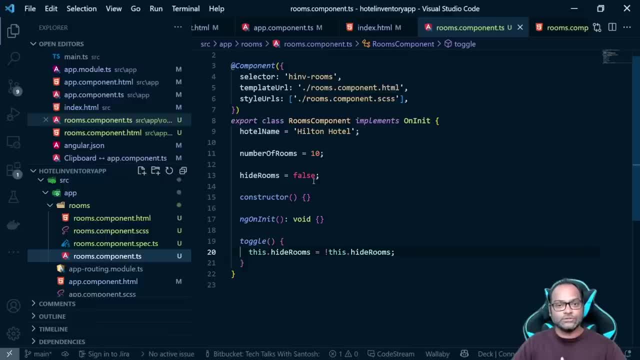 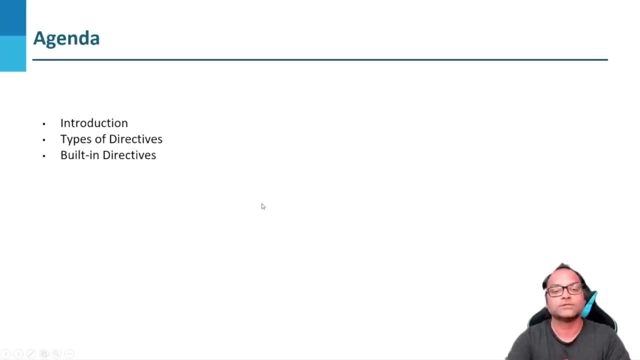 binding, you learn about event binding and this is what we are going to use for all our upcoming tutorials. in this video, we are going to talk about directives, so we will see types of directives and we will also see built-in directives. in this particular video and later on in this course, we will also 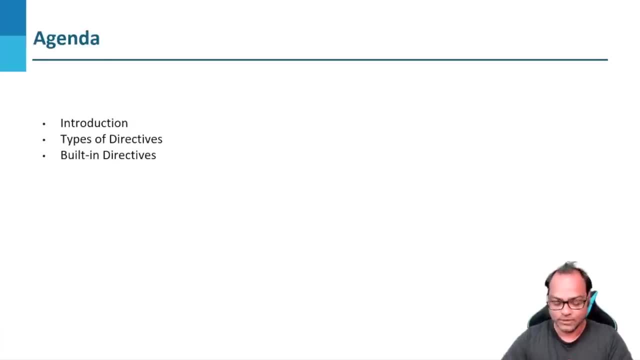 see how you can build your own custom directives. yeah, so let's go ahead and see what directives are. so directives are something which can change behavior or appearance of your dom element. they are kind of like, and you can say that they are a reusable function which you can apply on any. 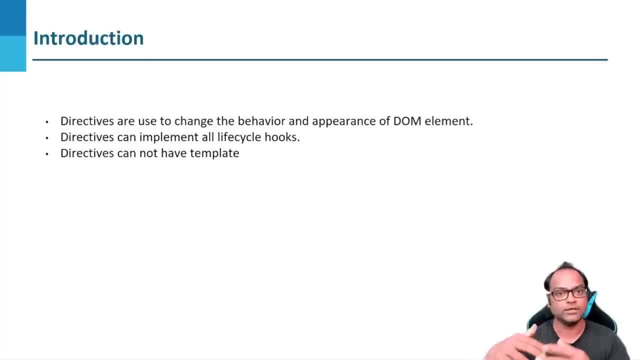 dom element which you have in your application, and then if you want to change that behavior of your dom or let's say, appearance of that dom, you can achieve that via directive. directives can implement all lifecycle hook. we have not learned about lifecycle hooks right now. it will be in upcoming videos. but just remember this: by implementing, you can also implement all. 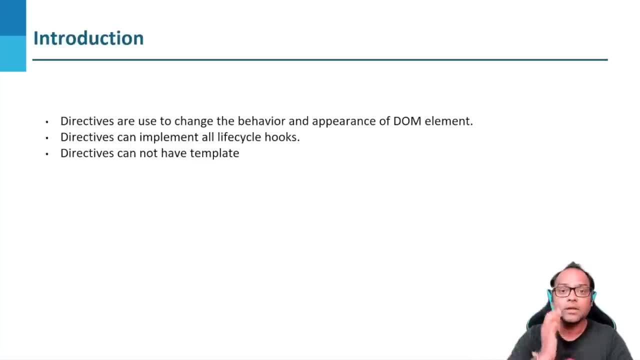 the lifecycle hooks, because we will be using that later on. the one difference between your components and directives are they cannot have templates. remember we, when we went through all the components, we said there will be four files every time and there was one template, one style sheet. then we have your, you sorry, your spects and then your ds file in directives you will be having. 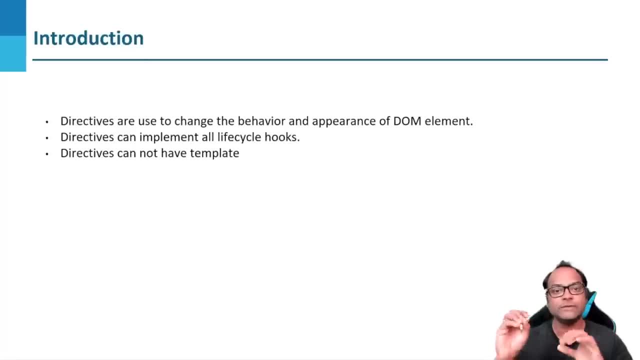 you won't be having a template file, so it will be just have your directives, will just contain your logic. so let's talk about types of directives which we have. so there are two types, which is one is structural directives and one is attribute based directive. structural directives are always 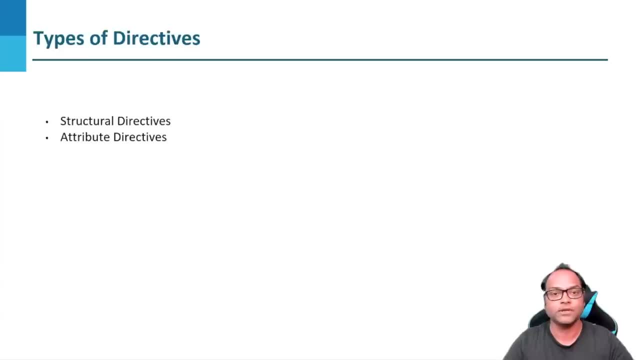 costlier because they are going to implement- uh sorry, structural directives are always costlier because they are going to change the behavior of your dom, which may give you performance- performance issues as well. attribute directives you will be using a lot of the time, probably most of the time, you will be creating your own attribute based directive rather than structured. 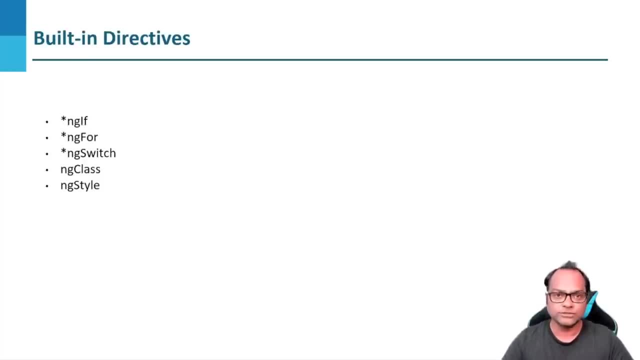 directive. so let's go ahead and use some built-in directives which we have available and later on, and we will also talk about what are the structured directives and attribute based directive which we have while going through each built-in directives here. so first we will, we will go through ng if ng if directive and let's see what we can achieve. 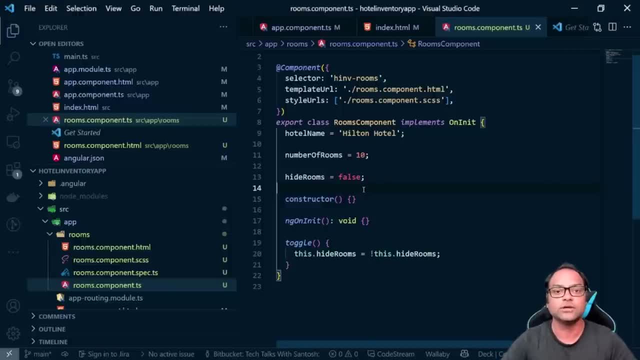 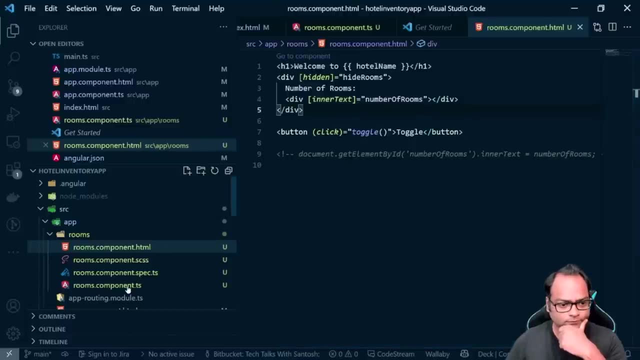 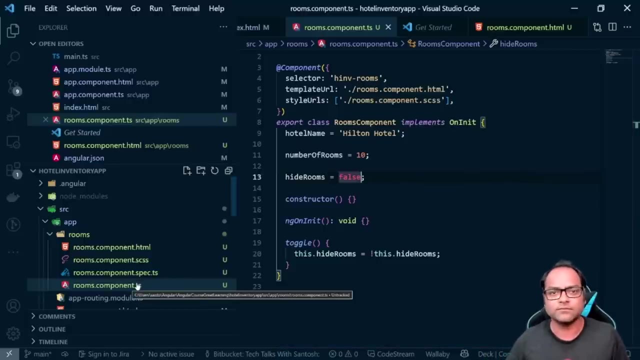 using ng if directive. let's go back to our code. this is our code here. uh, so, uh, what we will do is we will also, uh, we'll, we'll create one interface where we will have some, uh, information about our rooms. so let's go ahead and do that, let's create the interface. i'll call it as rooms dot es. 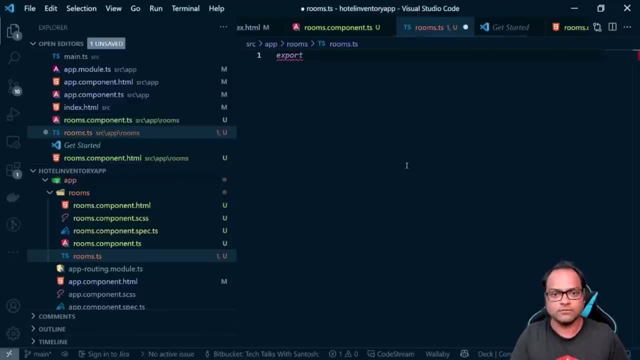 so this is our interface name. then we can say: export interface. remember the desktop session where we created our interfaces? and i'll call it as room and let's see, uh, what this room, uh property is going to have. so let's call it as room and let's see, uh, what this room, uh property is going to have. 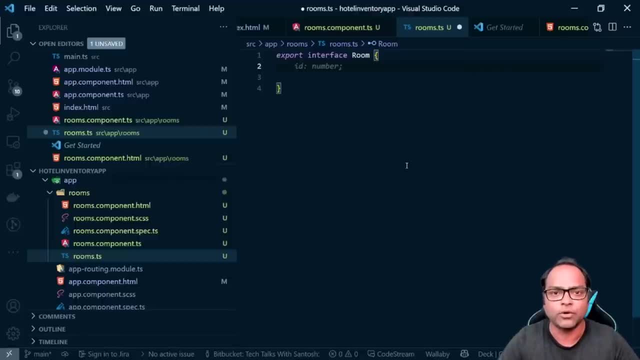 it will have, uh, as of now, we will. we will keep adding more properties as we uh go, but right now, let's say we have available rooms, which is number, then we have book rooms and uh, let's have these two properties as of now, and then we'll. 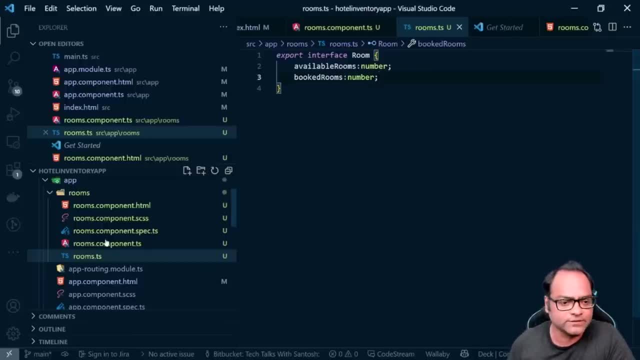 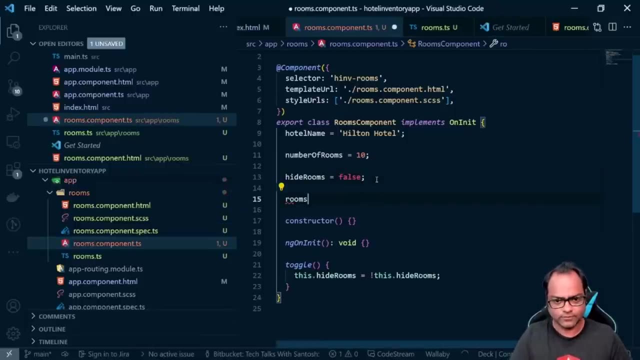 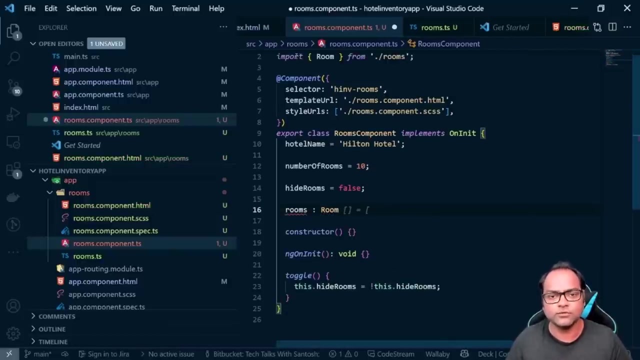 see later. and here i'm going to create a rooms property which will be type of room which is imported from. you can see. actually, due to angular language, service it auto- it can actually auto import out. this is something which is also enabled in vs code. so let's go ahead and create a room which is imported from you can see, uh, actually. 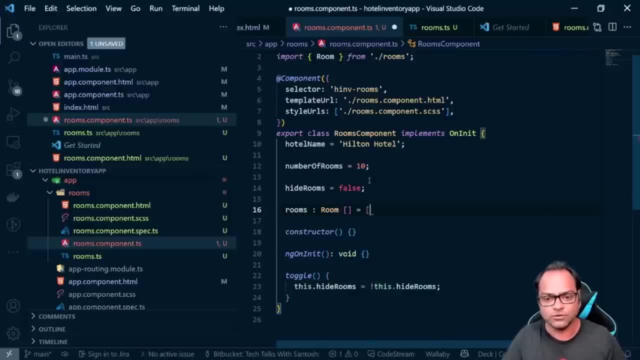 due to angular language service it auto. it can actually auto import out. this is something which you can just go to room and, uh sorry, it's not going to be array, it's an object, and here i'll say: available rooms is 10 and booked rooms is 5, and let's have 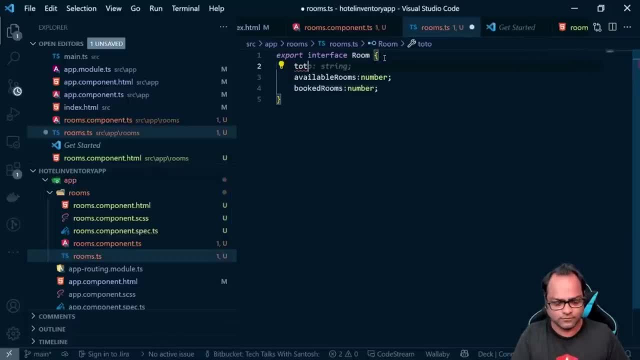 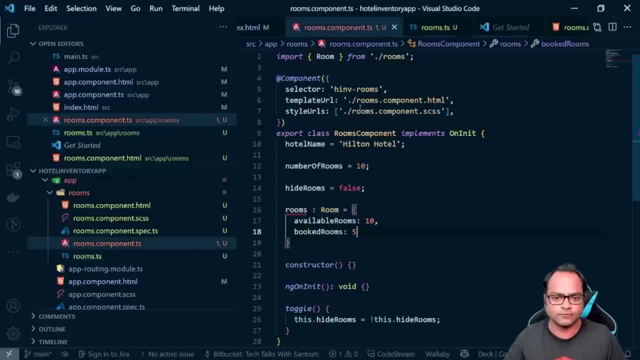 total rooms as well. so let's say, you have total rooms as 20, but you are just booking for 15, right? so where you have five available and five booked and five probably some something on hold or something like that, right or going through construction. so you have this now you, you have this data available and 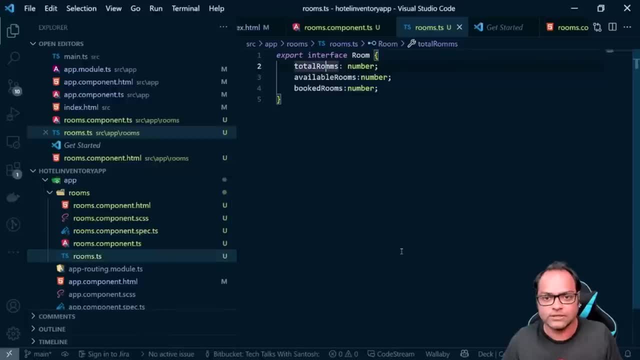 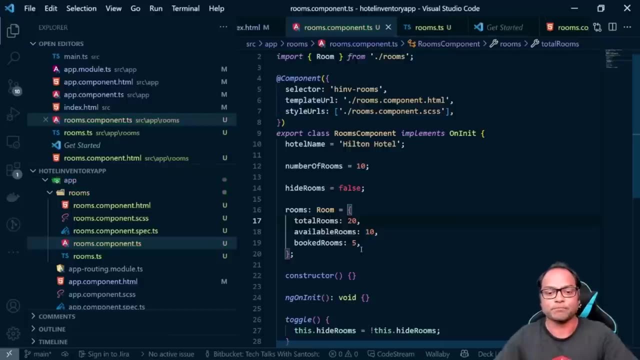 what we are going to do is let's first see in the spelling- i think i'm not sure why i'm keep misspelling rooms somehow- so you have total rooms, available rooms and booked rooms. so what we are going to achieve using this property is we will be using ng if directive. we will see an example of. 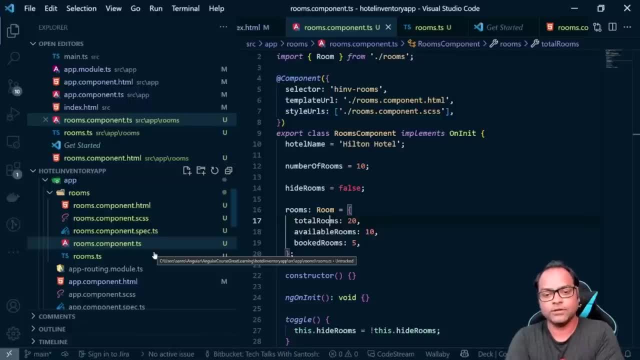 ng if directive and let's say, if available rooms is greater than 0, we want to display a section where probably you can see which which rooms are available, right list of rooms which are available in future. right now we don't have the rooms that are available right now, so let's just go ahead and 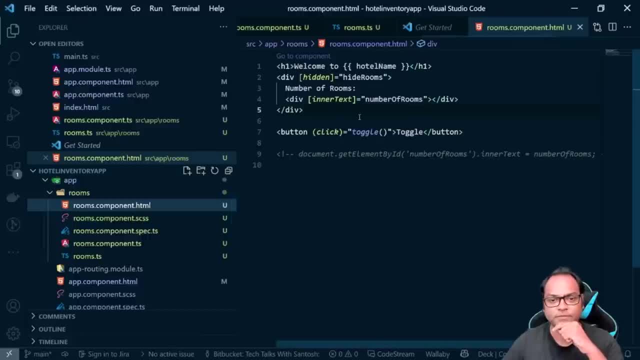 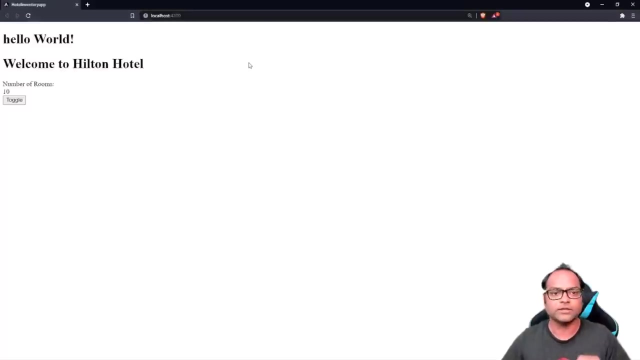 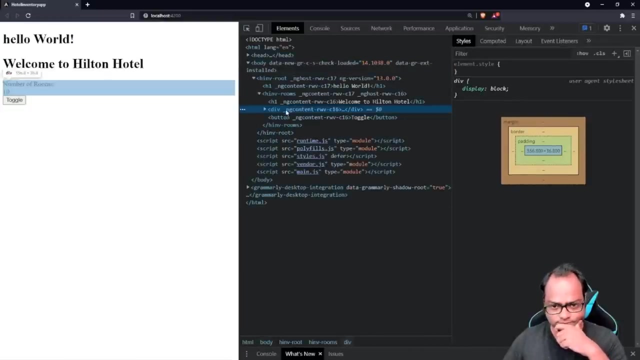 rooms list. so here let's see how we can achieve. remember, we said we can also use all the valid properties of HTML while doing property binding and we saw an example of hidden, but there was one problem with hidden attribute. so he. so the problem was, if you inspect this element and see this number of rooms and 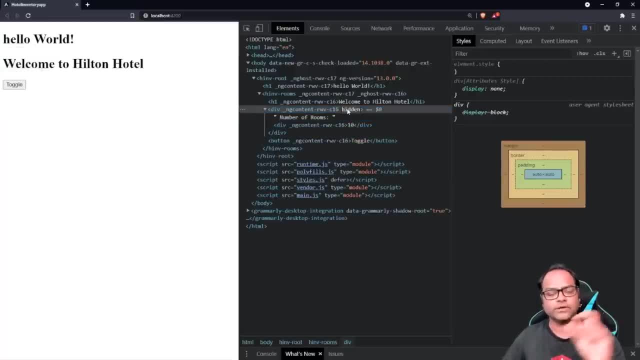 just let's keep toggle we. even though that particular div element is hidden, it is still available on your tongue. and when you have lot of Dom elements on your you, your view, it will cause performance issues. so what we can do. but in case I don't display this Dom element until unless I need it or I can just 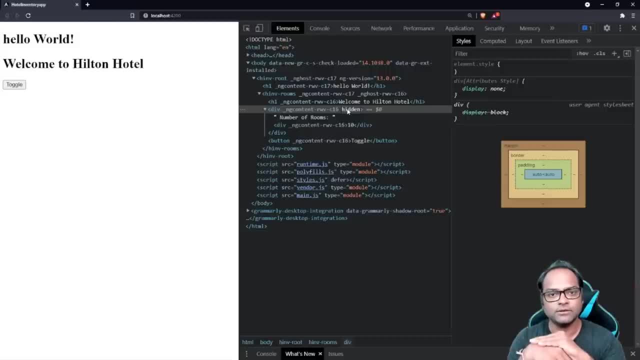 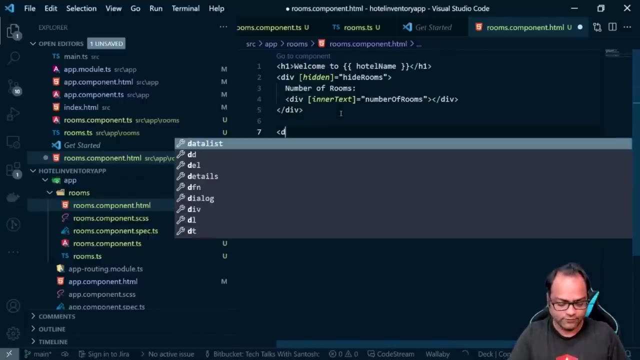 remove it whenever I don't have any rooms available. so in that case my dome Dom element will be fewer than then what we can expect in case we display all the elements. so let's go ahead and try to achieve that. so I'll create a new div here and here. 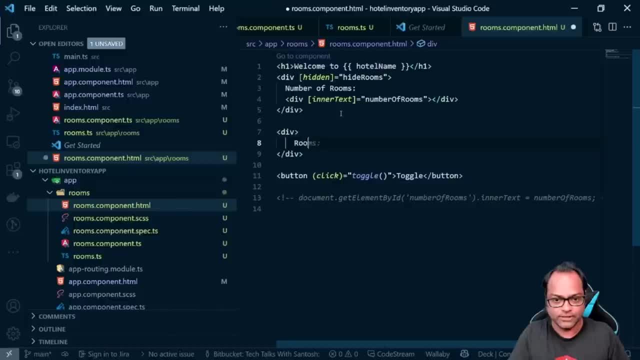 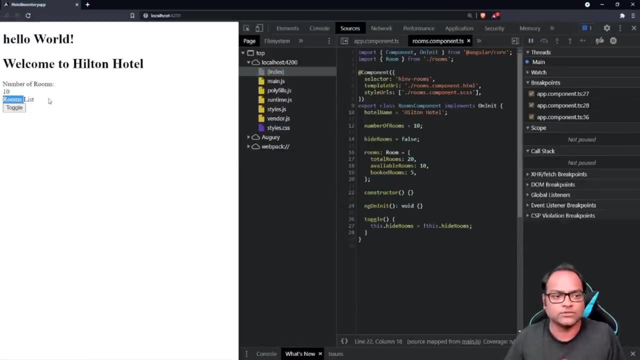 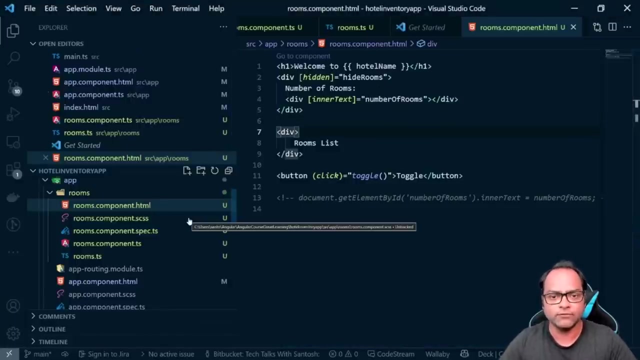 I'll say, for example, I mean going to display rooms list here in future. when we have room list of rooms, let's see if, okay, remove this breakpoint first and we get this rooms list. now the case is, in case rooms are available, I want to display this entire thing. I mean, I can have anything here, right, I can have a. 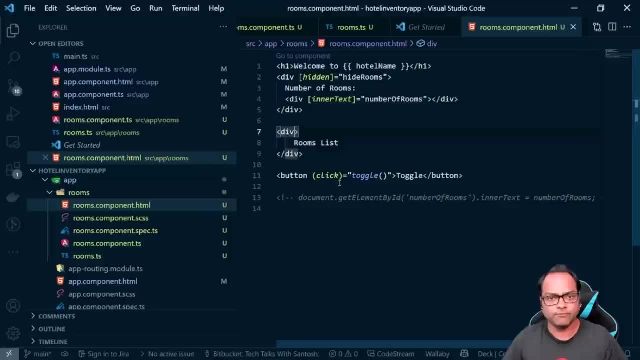 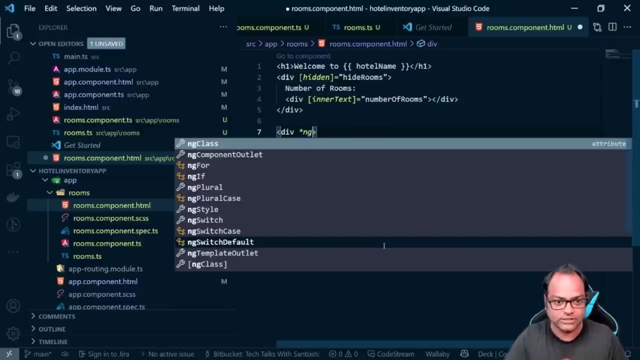 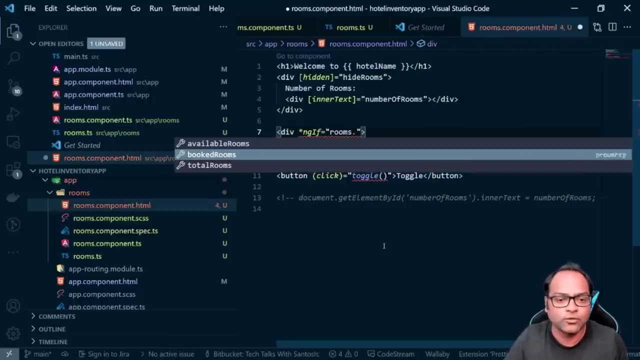 list. I can have whatever I want to. in future we are going to have list, basically. so here what we will do is I can just access this rooms property here and using the ngif directive- so star ngif if is equals to- I can say rooms dot total available rooms. 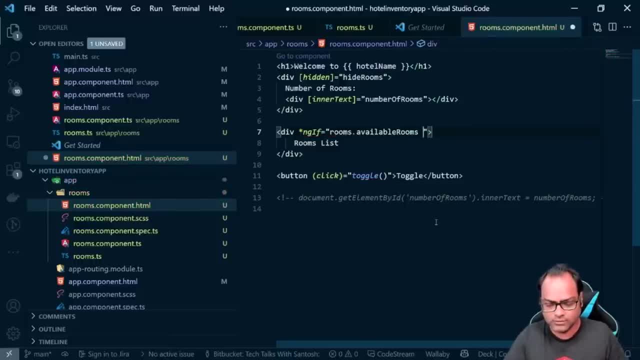 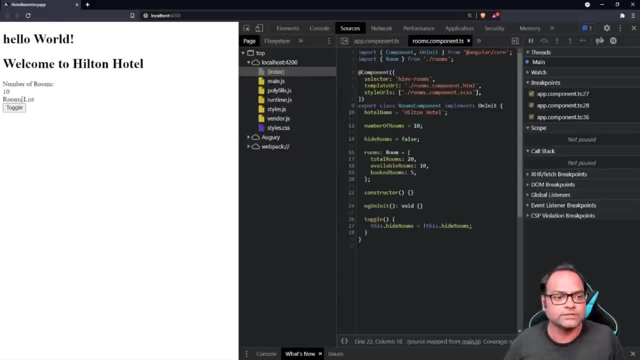 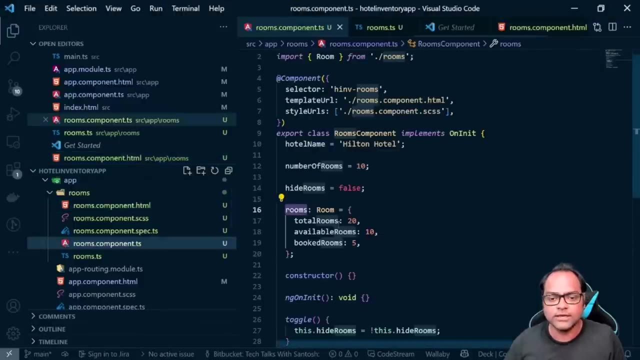 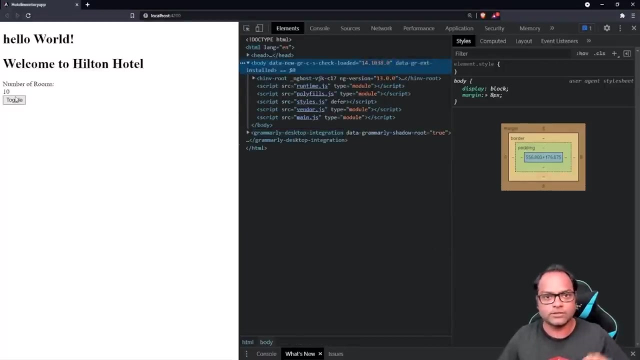 if it is greater than zero. I want to display this so rooms list right now. of course, our available rooms are greater than zero, so we will get this rooms list and it is available here now. let's go ahead and change the available rooms to zero and let's come back here. okay, so that particular div is gone, but let's inspect. 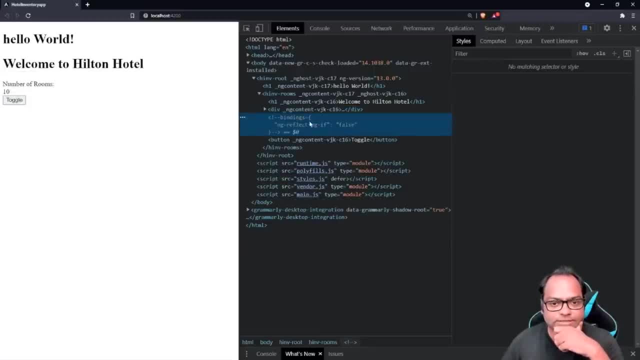 the element. this is, this is where it gets interesting- right so you can see that div, entire div, is gone. it's not available in your DOM. so something which, let's say there are some, some secure information which you don't want to display to all user, but let's say you want to enable that particular area or 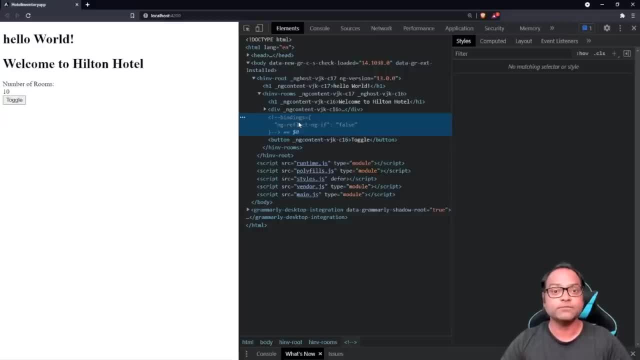 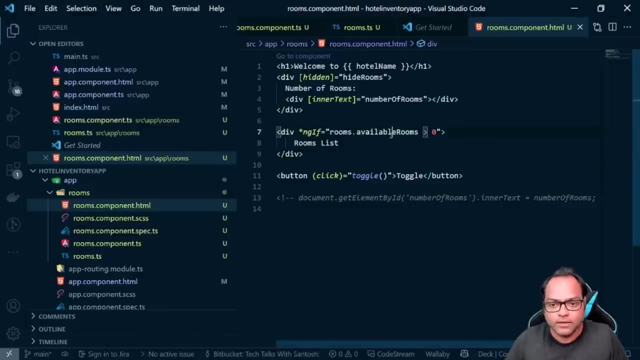 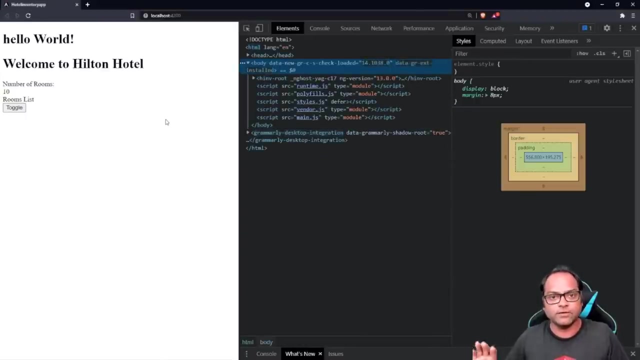 you want to display that particular section in some particular case. that's it. you have the perfect use case for ngif. try to use ngif as much as possible. don't rely on the hidden attribute. so that's one thing. now let's go ahead and change this to then. so we have learned about ngif directive. 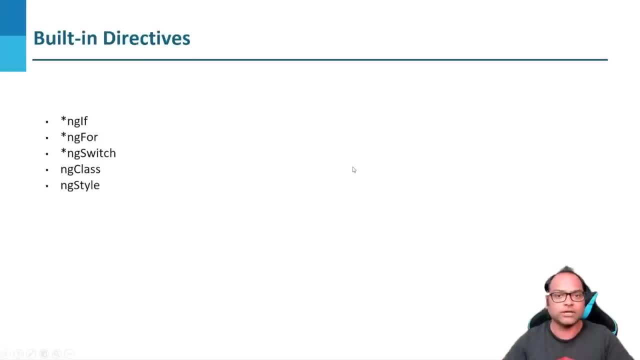 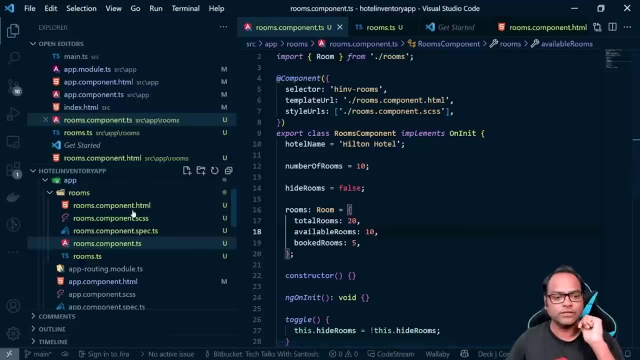 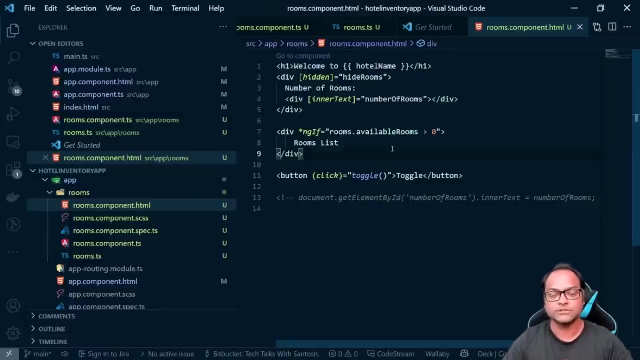 now let's, let's go ahead and see what are. what else is there? so we have ng for okay, before we go to ng for right i'll. i want to show you some some more. i can say syntax which you can use. so here in a typescript, this is something. this. 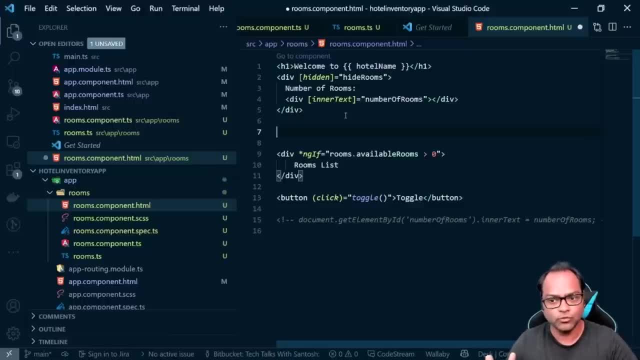 is known as optional chaining and there are two, two sorry. there are two features which are actually enabled in type script, which is optional chaining, and null knowledge question chaining. this is where we are kind of like we are testing if any ways that there there are two words. here let's say this was the type script, but thecondash is about to appear, something we so let's see here. so we open a function. it sort of sounds like fundamental itself. so this is Skilled. 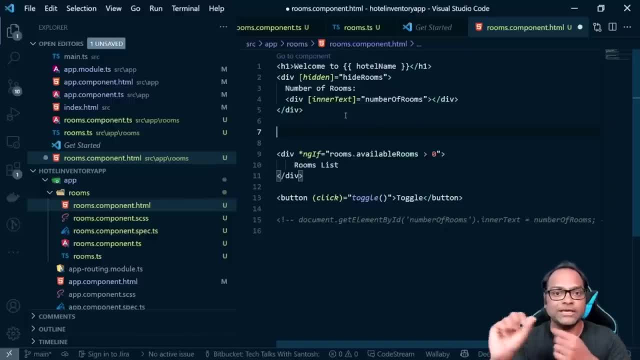 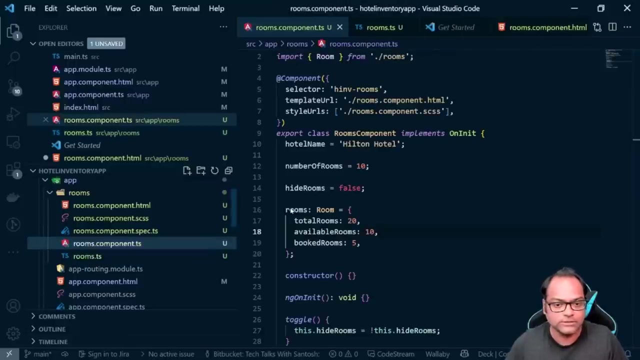 collision, collision. you can actually use both inside template as well. let me show you some example. so let's say: if my rooms, my rooms property, right, if my rooms property is not available, what i can also do is i can say no rooms, so let's see. so what i will do here is i'll say: rooms is this, and i'll just 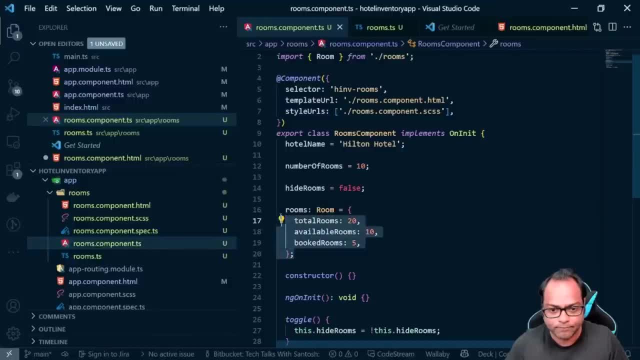 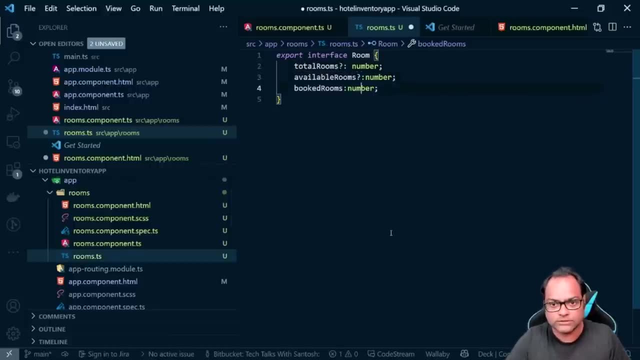 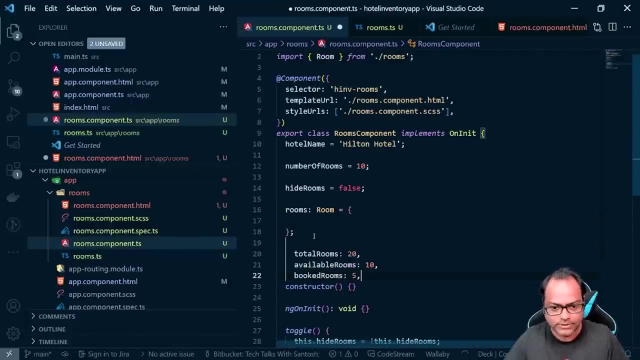 i have to make it optional. let's do that quickly. so, question mark, question mark, question, and i will comment this. i'll keep it here so i can now. we can go ahead and use it later on. but let's see, so we have. we don't have any uh data available for rooms. 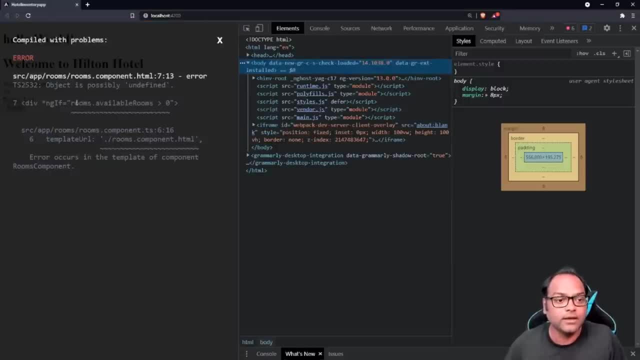 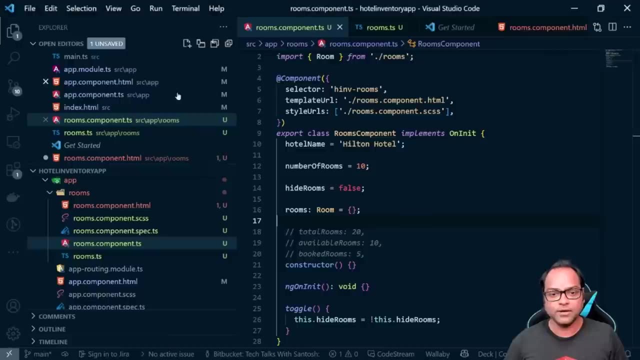 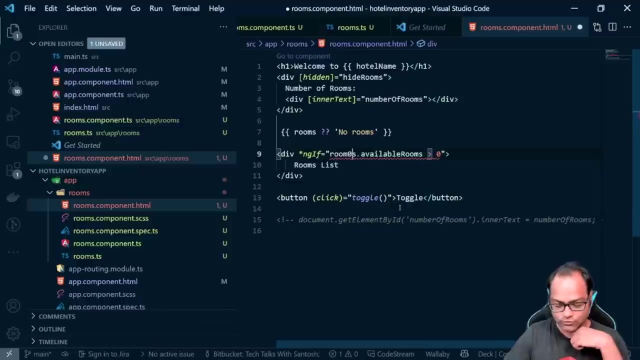 let's see what we get here. so we are getting an error. so it says rooms dot available rooms is greater than zero and it says object is possibly undefined. what, in this case, now, what we can do? so of course, this will be taken care by an alish pollution operator, but you can also use the optional chaining here you can put: 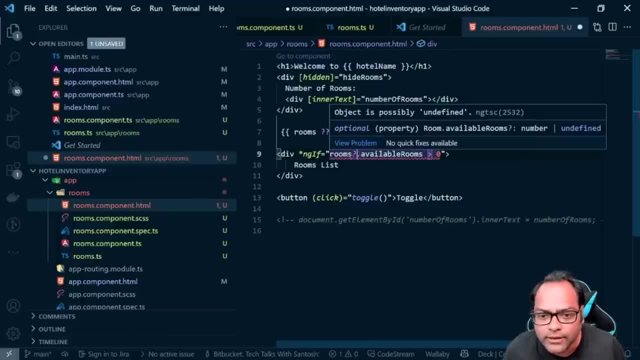 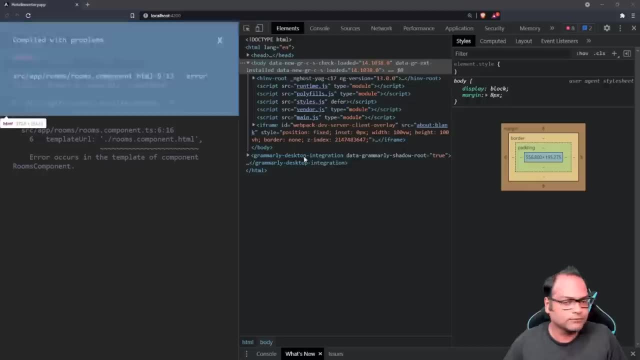 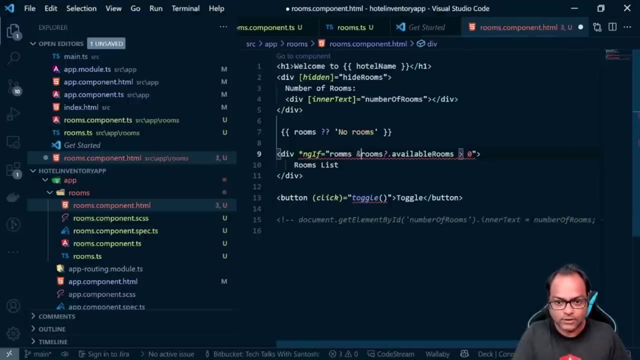 a question mark and let's see- oh sorry, i can do some rooms- and if rooms and rooms dot available rooms is greater than zero, let's see it works. let's see it works. uh, uh, let's see. uh, we have made some changes, so we are saying rooms, not available rooms. so, in case, 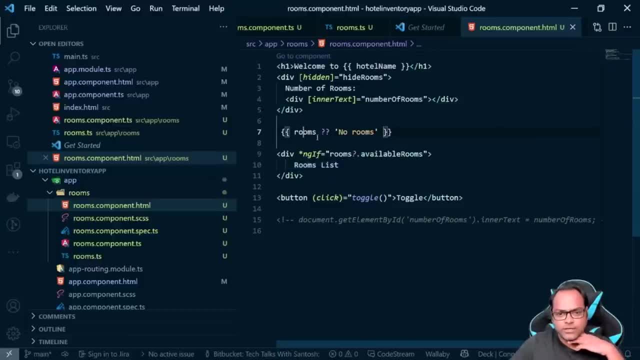 rooms is available, we will display rooms list here. let's see what it displays. okay, it is showing object object, which of course makes sense because we have to change, uh, we have to check for an individual object, right, and so here i can say i can just use the same. so i'm saying, if uh, 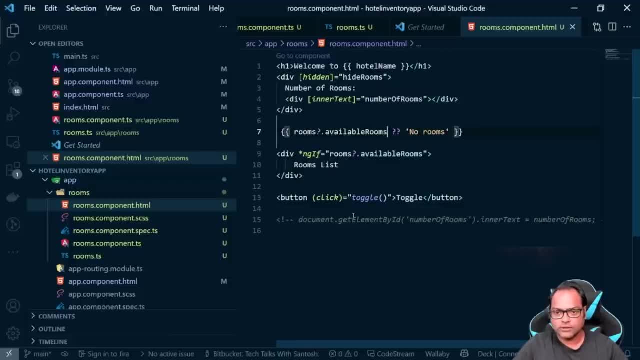 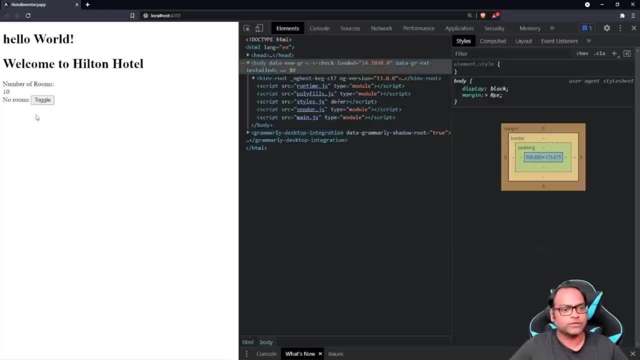 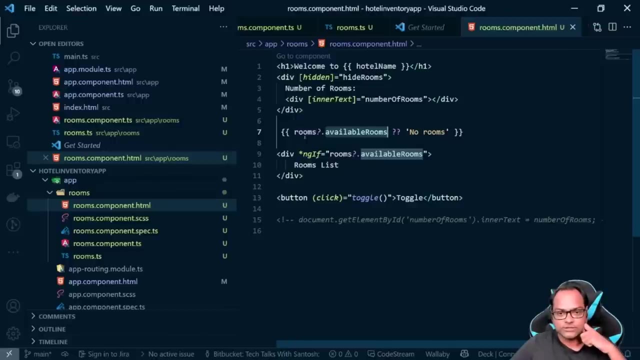 rooms not available. rooms is available, then, uh, it's okay. otherwise, just go ahead and display no, no rooms, and it should work. yeah, so you have no rooms available. in case there is, uh, the available rows, available rooms does not exist, so this is something which you can use. uh, which is null. 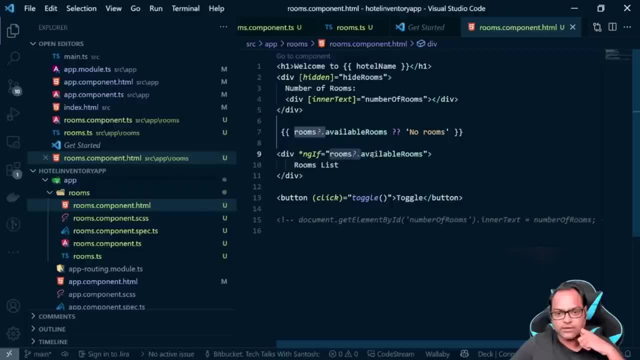 collision operator, and this is optional chaining, so you can say, okay, before accessing this variable, go ahead and check if this exists or not. so this is really useful. in case you want to bind some object, you don't have to worry about it, i mean, uh, whether this object exists or not. so we generally 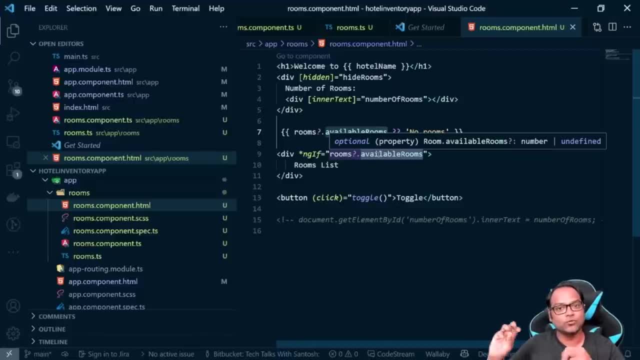 do right if and else that, so you don't have to do if and else. here you can just put a question mark and try to access an object. if object exists, it will print it, if doesn't exist, it will just leave it right. i mean, for example, this rooms list- right now available rooms- does not exist, so it is not. 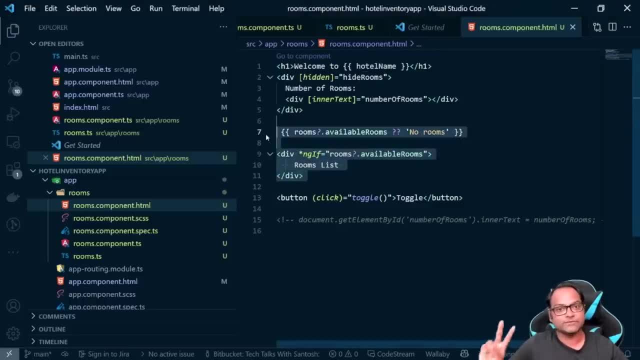 displaying room list. that's it. so these are two operators, which is really useful while working in angular template. they are available inside your typescript file as well, so feel free to use them there also now once. uh. now we know about these operators and we know about ngif. let's go ahead and do some uh. 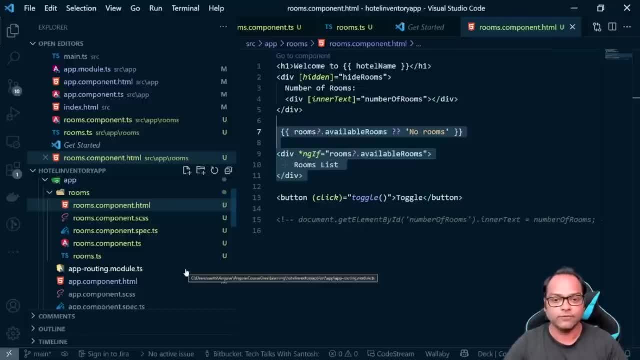 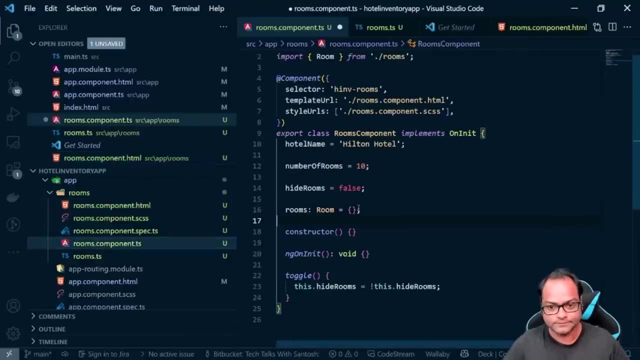 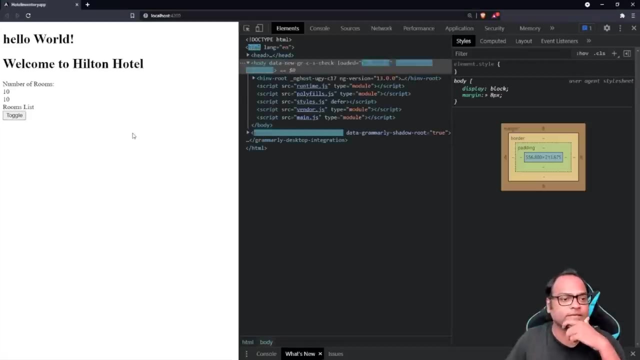 extra stuff, right, so rooms list. we said, uh, we want to display rooms list in case we have available rooms. now let's go ahead and put this code back. let's see, it breaks the template, it doesn't. so we we still have rooms list and it displays the. 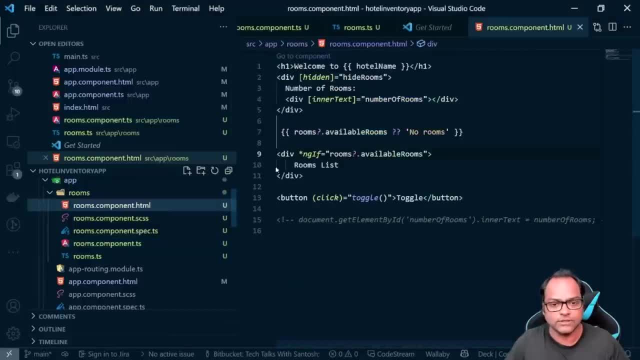 number of rooms which is available. so which is this, this line of code? so, rather than this div, i could have just used this, which will take care of- yeah, i mean, in case my rooms does not, uh, there are no available rooms, it will also show norms. so let's see this: available rooms is greater than 0. object is possibly undefined. i can just 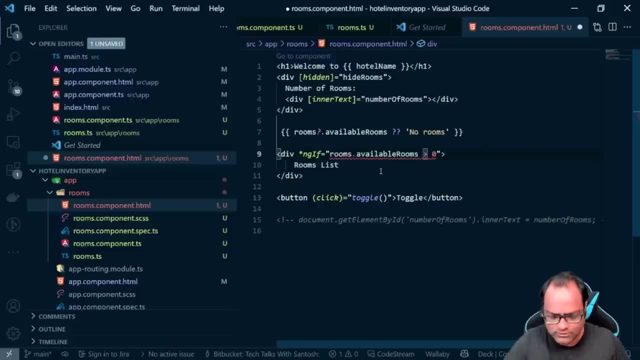 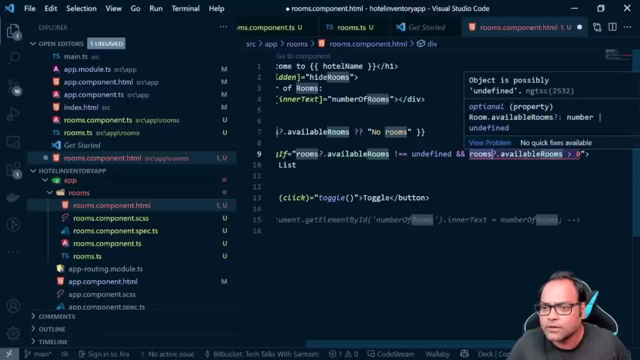 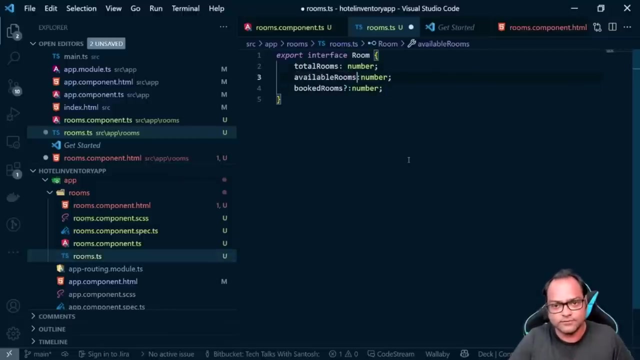 remove. let's see roomsavailableroom: okay, do I need to check if it is undefined? let's see, not mean this part. let's see: hmm, so available rooms not equals to undefined and rooms- okay, I'm still getting this- that are somehow because of this question mark, which let's remove it. 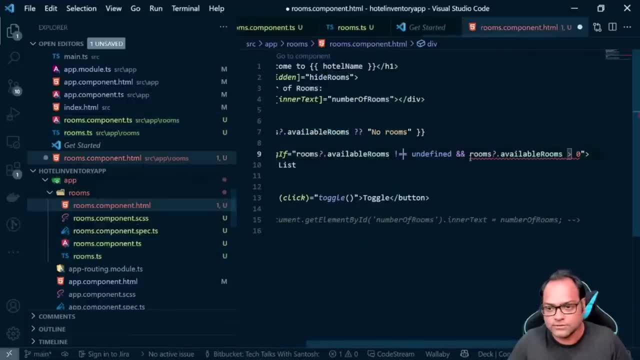 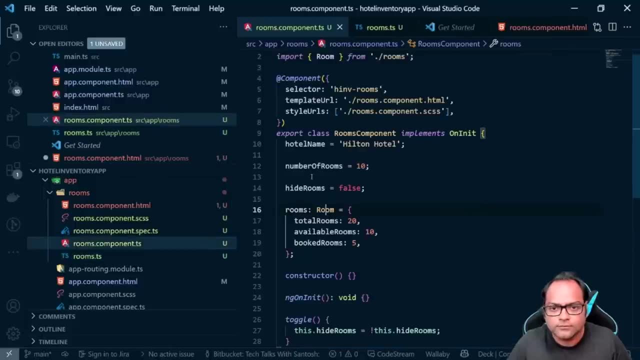 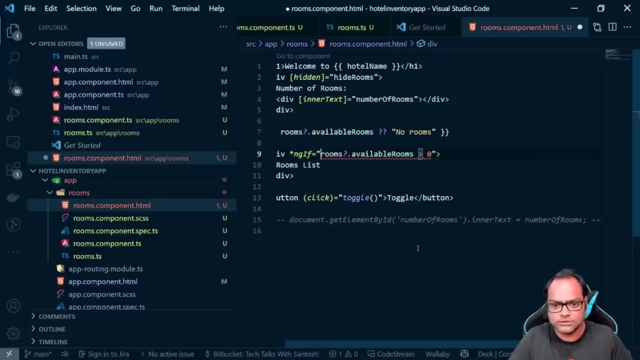 which make it makes the value as undefined as well, so you should not be getting it anymore. numbers HTML: okay, this strange rooms, not available rooms greater than zero works, so we have like our. now we want to display here rooms list. now we need rooms data, so we need rooms list. 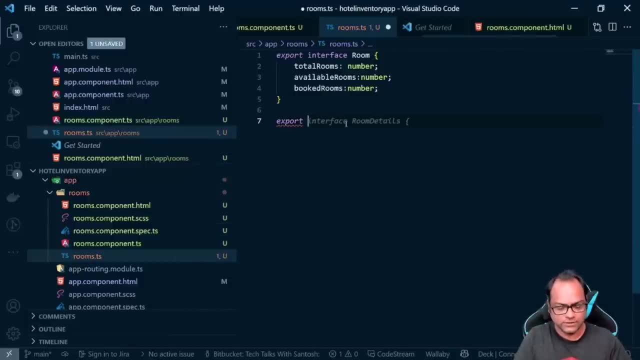 data. so what we will do is we'll create an interface and we will call it as room list. let's add some property. so first thing which we will do is the room type, right, so you can have it. look, there are multiple room types, which is, let's say, right now, string, and what else we can have. but I don't can. 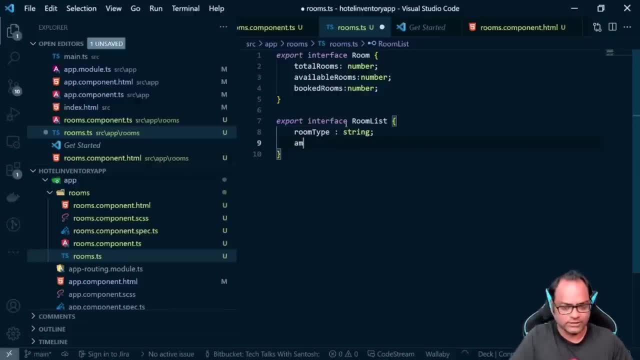 have amenities, right. we will say: this is amenities, which is sets up now. string then the price of this particular room, which is number and what else? what is a room can have? uh, it can, of course. amenities is the their room type is there. it can have an image, right? so photos. 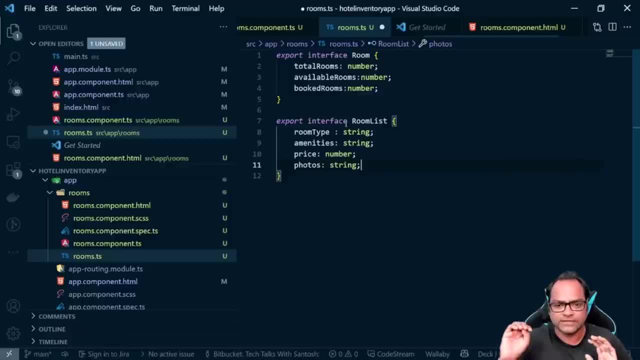 which is uh, which can be string, uh, area of string, but let's, let's say we right now we have only one, one photo, so this is and uh available one one day time property as well, so we can have checking time right. so we will also have one day property and checkout time. so we have string number date. so, yeah, i think this is enough. 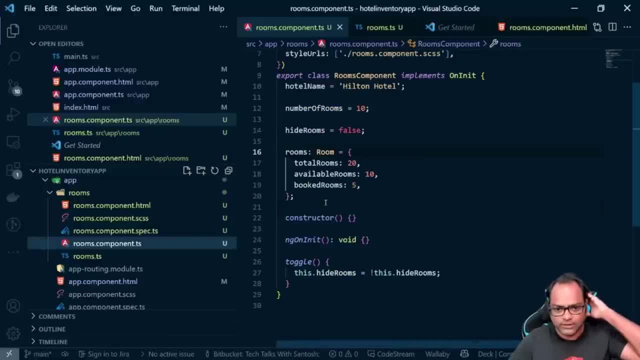 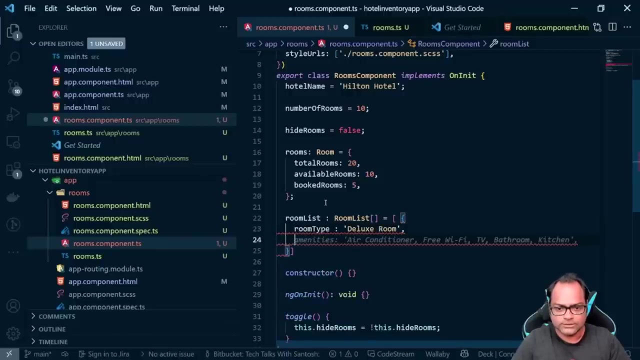 this is more than enough information. now let's go ahead and create some data. so i'll say room list, let's just type of room list, and uh, this is going to be added. so we'll just, and let's say room type, uh, amenities, price, and then we have. 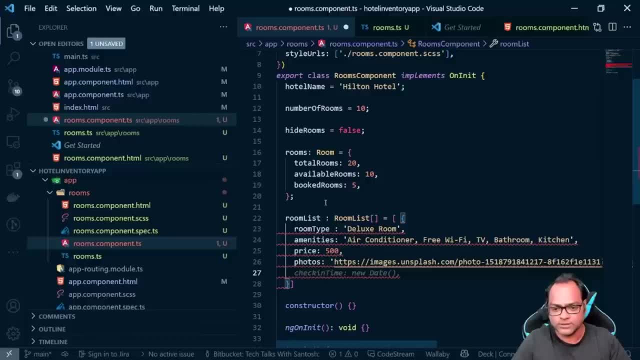 photos. let's take some something from uh unsplash check-in time. let's say we have uh. let's put some date- uh 11th, 11th november 2021- and check out time this and we have to say new date and then in your application just try to use some uh date time from daytime, uh library, for example. 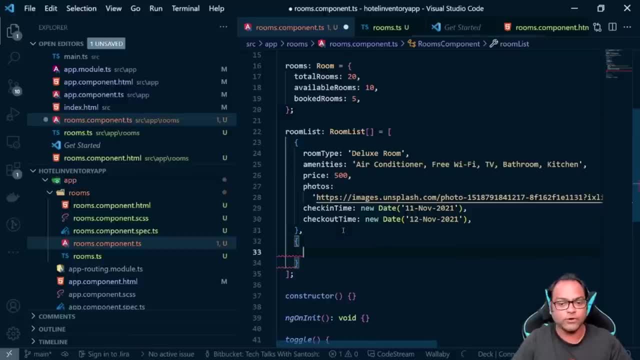 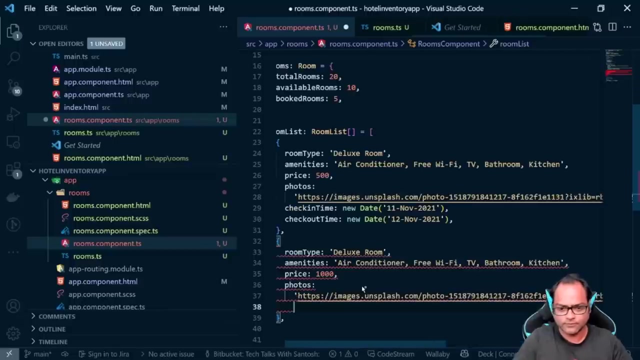 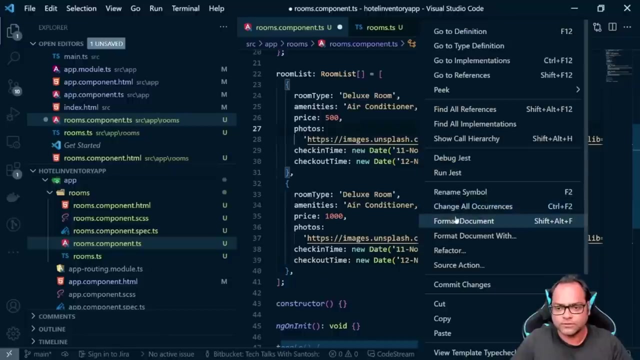 let's take date fns, whatever your uh you have decided for your application. so amenities price, let's say i'll just increase, to increase to thousand photos. let's take the same photo as of now and then we have check-in time and you have check out time. so 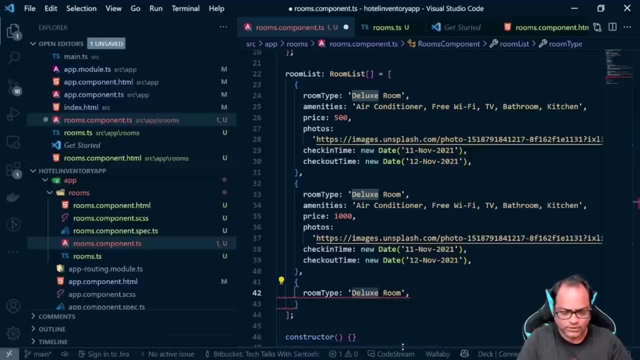 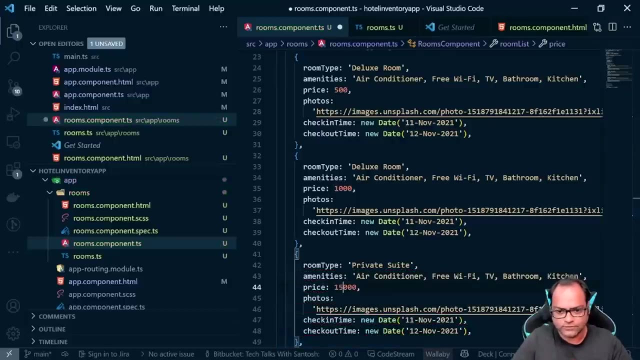 and this won't be deluxe room, but let's say private suit, and rest of the things are almost same. let's increase the price to 15.. okay, so let's go ahead and create a private suit. okay, so we have this list of records available here. now let's try to bind it. 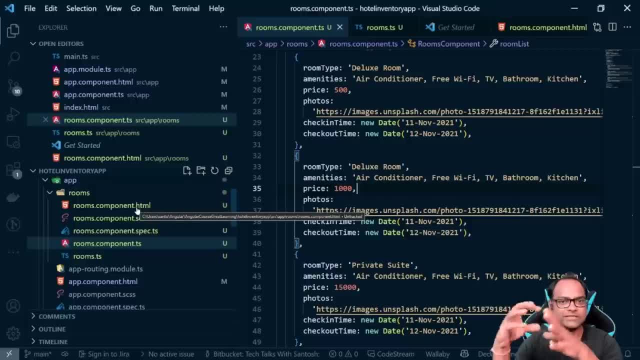 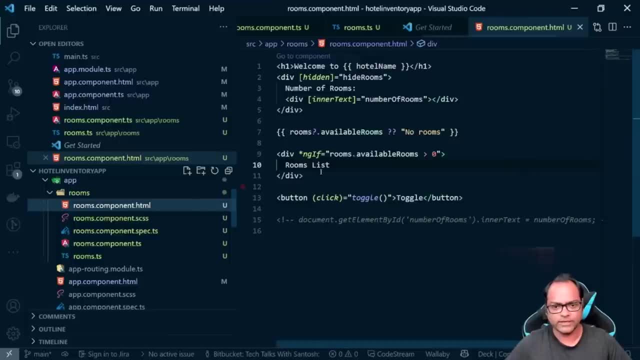 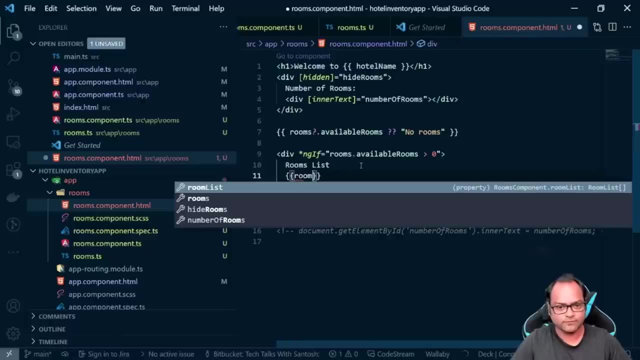 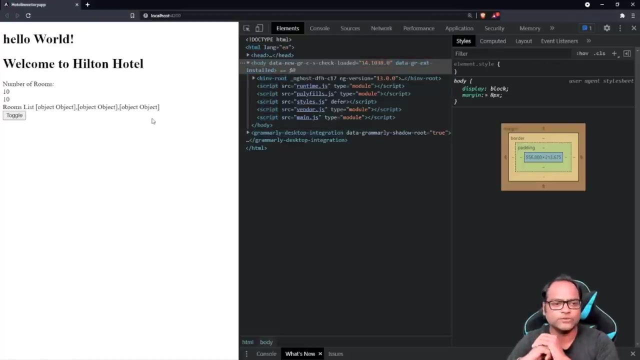 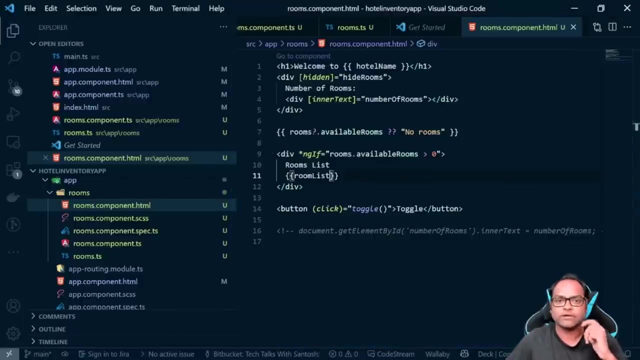 now we know how to bind values like string, number, boolean. we also know how to bind objects now. but what about arrays? so let's try binding areas here, right? so rooms list. i can say rooms list, so just let's place it here as it is. i'm bound in such a way that in this case you can't let the 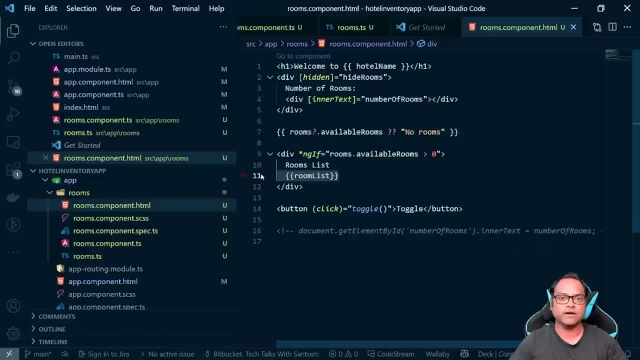 and copy it. we want to. So, generally, how you display area of information right on your webpage. If I have to talk about in HTML, probably we'll be using some data table right. So right now let's use tables And in future what we will do is we will remove this table. 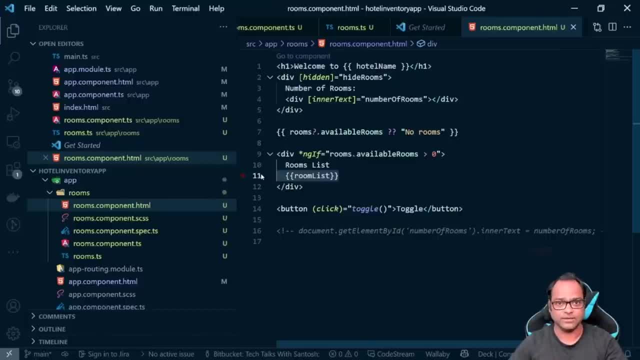 and we will use something from third-party UL library, because in your real-time project you are not going to create table, probably never. You will be using some UL library, so you should learn about that And that's what we will do in probably in upcoming video. 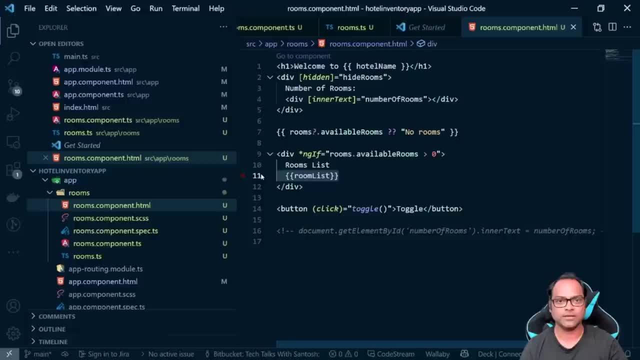 where we will remove this table and then we'll replace it with Angular Material Table. Why we are learning it right now? Because Angular Material Table will actually avoid, or you can say, it will give you a wrapper where you don't have to write this code. 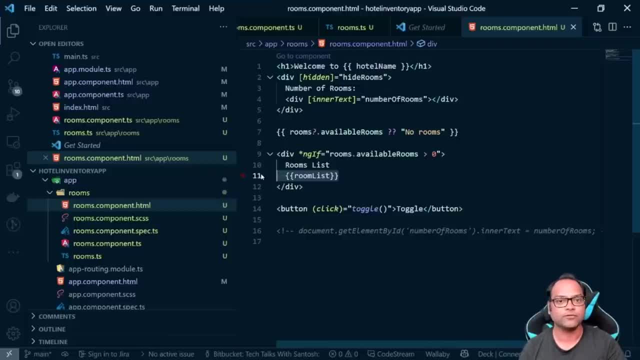 So you should learn about ng4 in case you have to work with area of records. But, as we said, Angular Material Table takes care of everything, So it will do internally all those things. You won't be actually writing this code, But this ng4 directive will be useful. 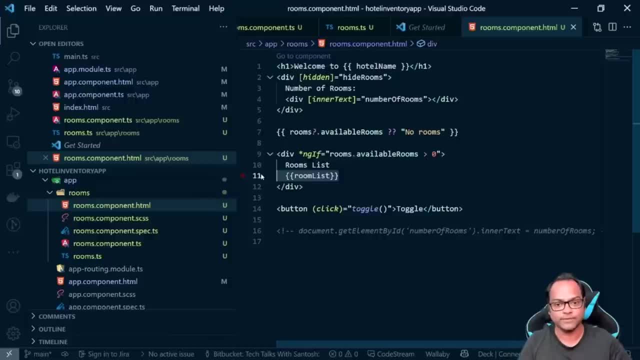 for a lot of other cases where you have actually area of data and you want to bind it. So let's use table And we'll say: okay, first there is a tr and then th. We have room number. okay, not room number. 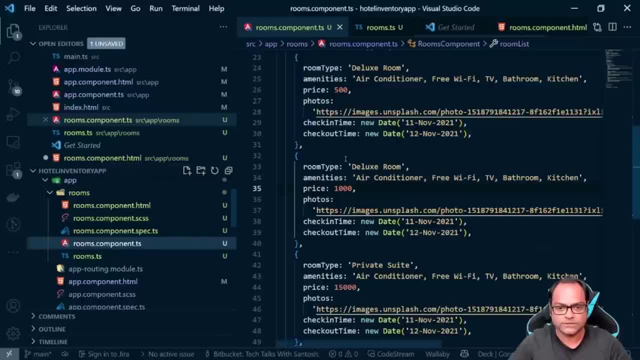 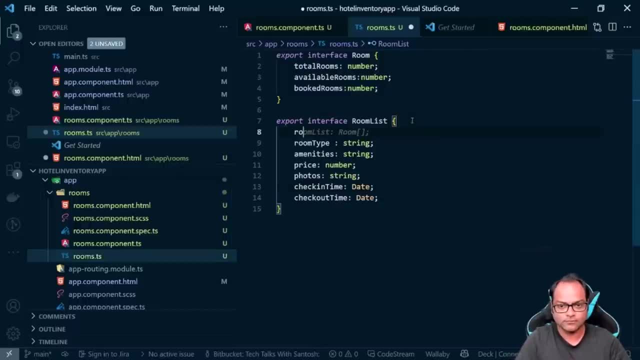 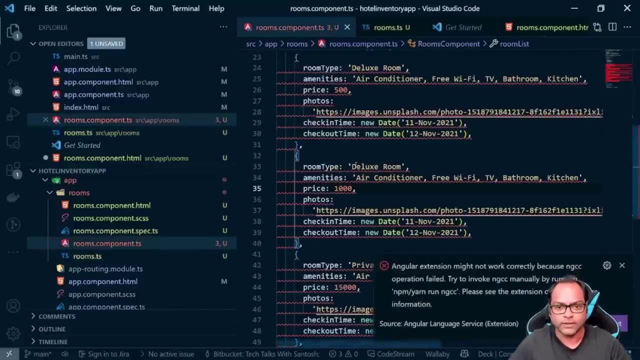 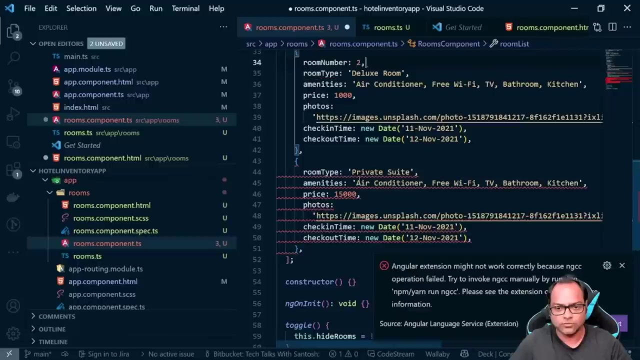 but we have, okay, the room number can be on property, which we missed, And let's add it here. So we'll say room number one, room number two and room number three. Okay, so we have our room number, property as well. 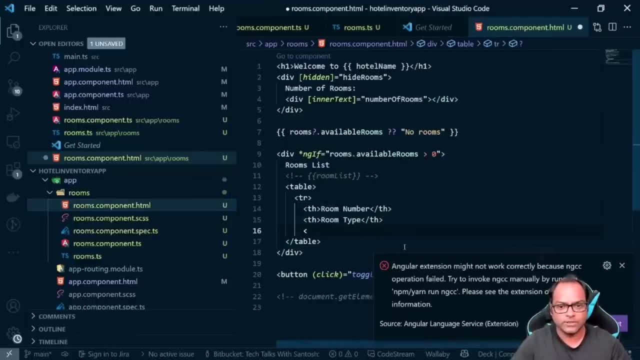 So let's see, So we have the headers, So we have room number, room type, then what else? So this will be our table headers, room price, Then we have room status. We don't have, but let's say we will have amenities, right. 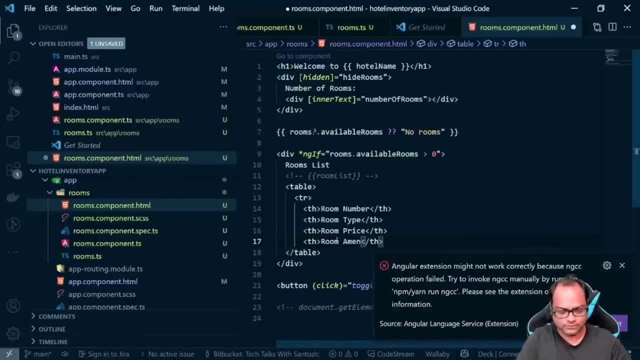 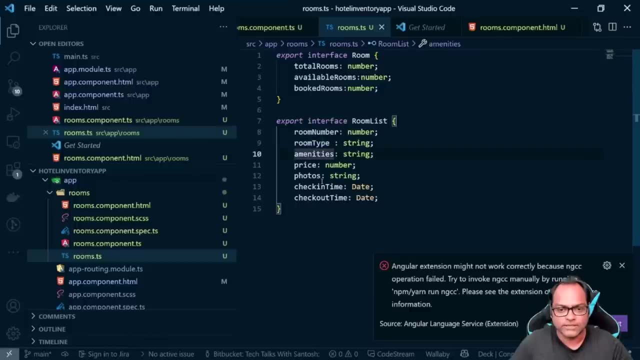 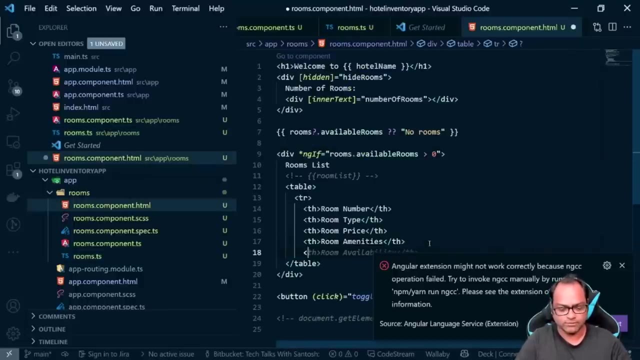 We have amenities, So we have room number, room type, amenities, price. is there Photo we will use later on Check-in time, check-out time, because we want to actually see some date time pipe as well. I'll just talk about it later, let's see. 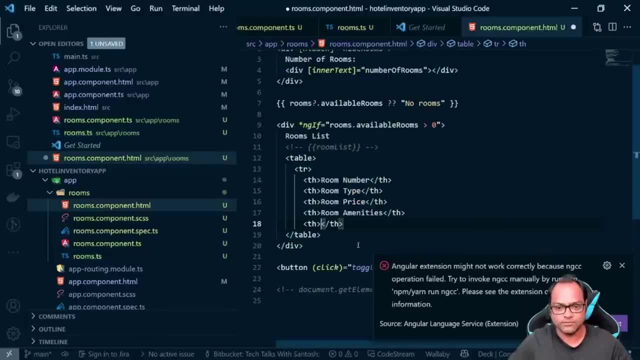 So right now, let's display this check-out and check-in time. check-out time, Check-in time. So let's use only one check-in time here. This is it, So this is our header, And now we want to display the information. 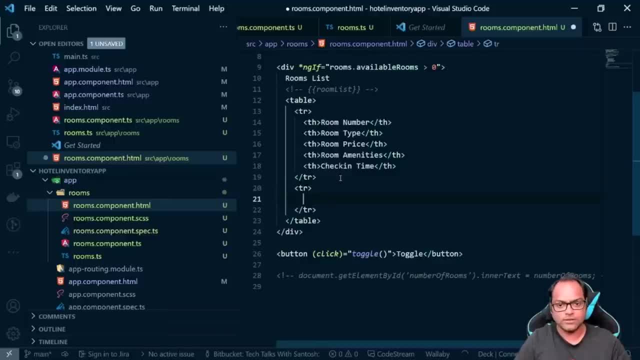 So let's come back here and have another TR, And now we want to. what we want to do is we want to create multiple rows, remember. So TR means, of course, your table rows, which will be created for each and every record. 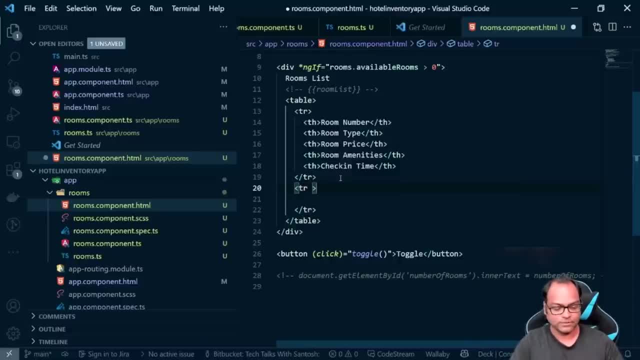 So this is where you will be applying your ng-for. So I'll say, okay, this is ng-for is equals to: let's see how the syntax is. So you can say: let room of rooms list. Okay, what happened here? 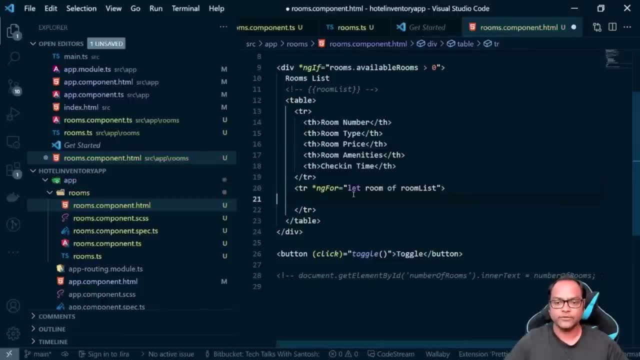 Okay, it's not rooms list, it's room list. Okay, so now this for loop will run for each record inside room list. So we have three records right now, And now let's display the information. So we have room number, type, price. 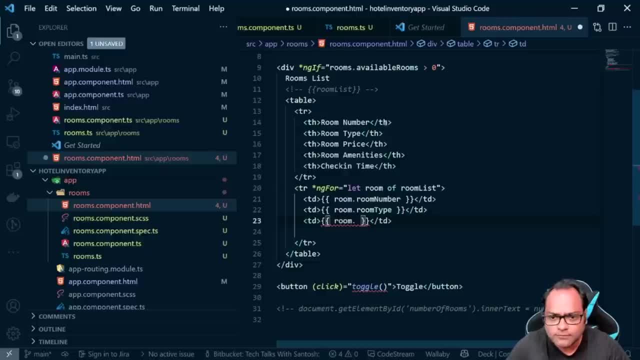 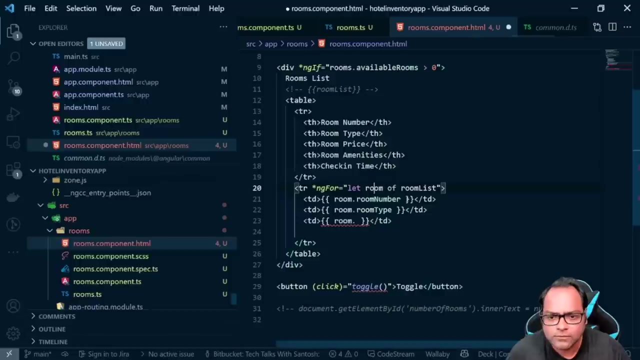 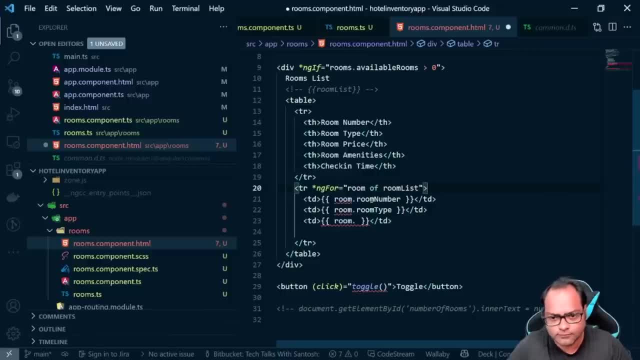 let's say next. let's say next, and after comment we'll see whether it's a good fit. What happened here? So we're actually not going to change any of our parameters. So what we're going to do is just go back here. 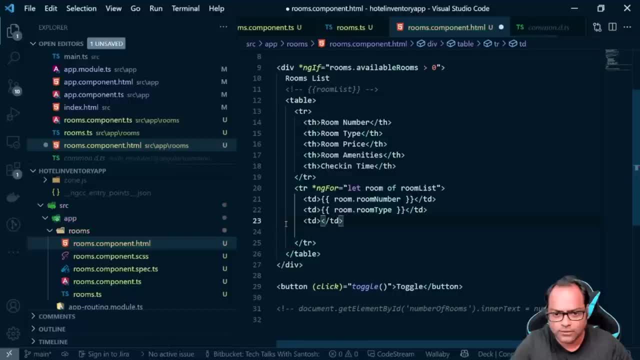 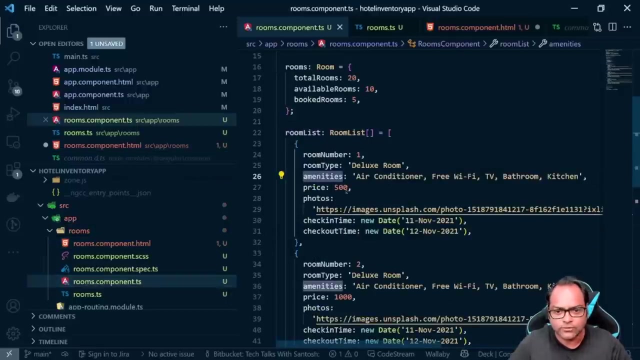 and look at everything in here. Okay, so now we have our data here And then we're going to go back here and look at everything, So we should get intelligence, but somehow the intelligence is not working. Okay, So we have price. then we need amenities. copy the properties right now: amenities. 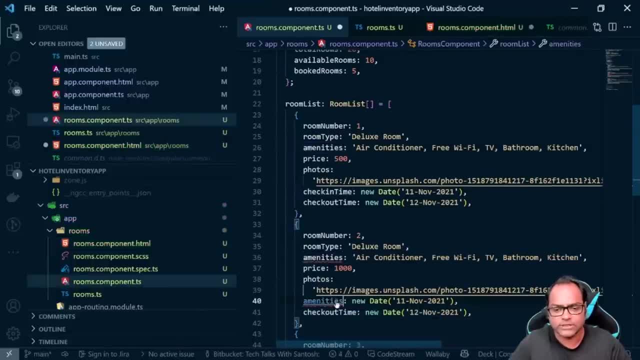 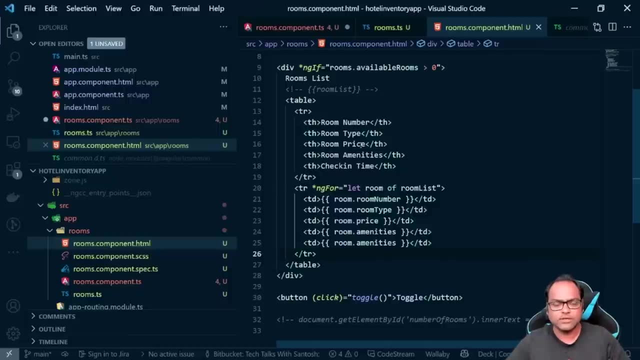 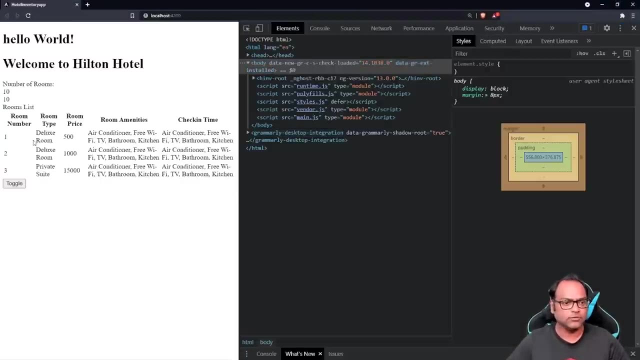 and then we have check-in time and that's another property check-in time. Okay, So now we have our room list available. Let's go ahead and see that on the UI. here you can see all the information is available in a tabular format. 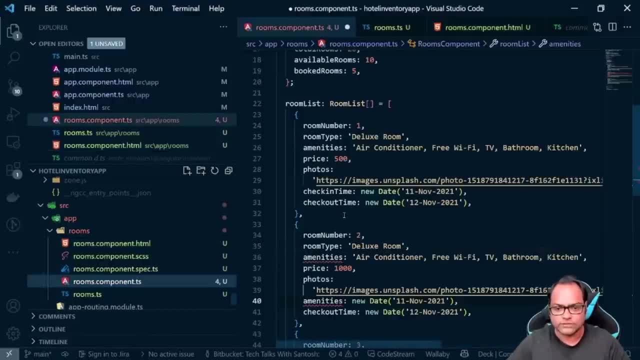 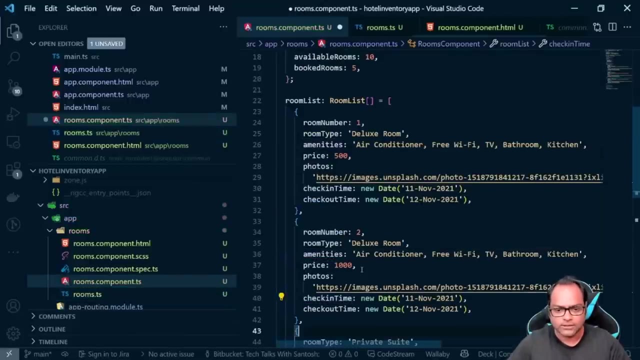 So I think, check-in time. okay, we have to change. it is what happened to this. it is not a simple amenities. Did I change something here? amenities, amenities. now there is a string. okay, I think I just. 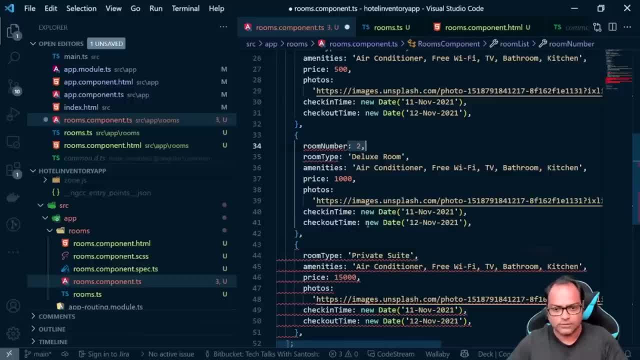 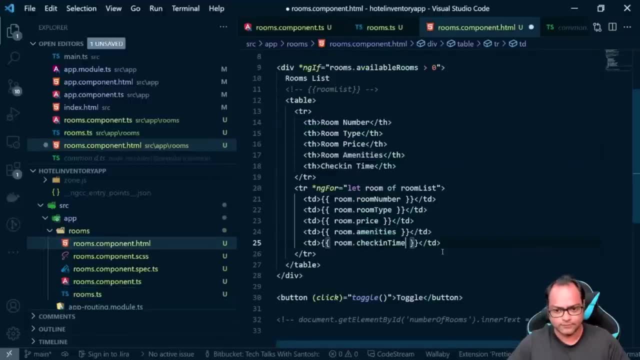 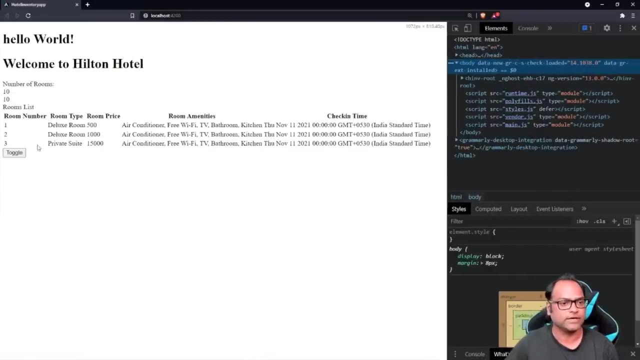 copy, pasted something, So check-in time which will be here. so let's go ahead and see the UI and this is the information which we have available in tabular format. So we have a room number, we have room type, we have room price. 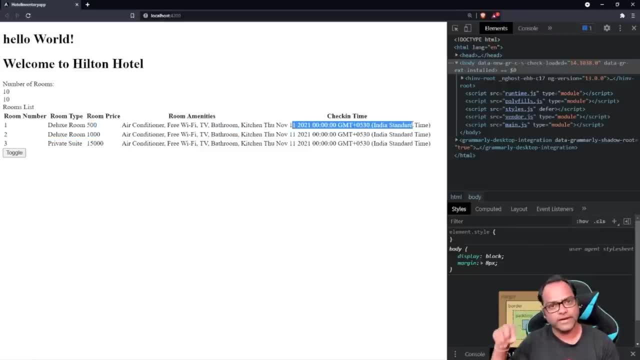 Then we have amenities and then this is your date format. So by default you can see, Angular display is the long date format which we can change. we will change this date format later on. Right now let's go ahead and see what happened here. 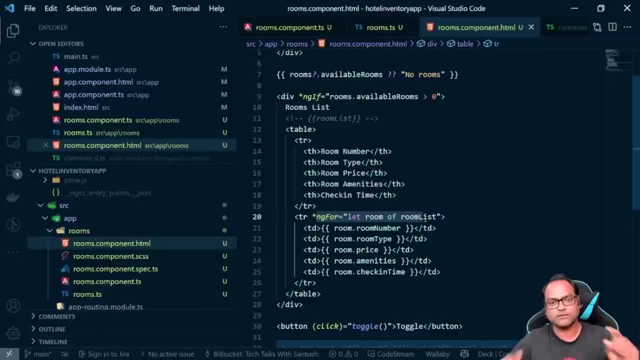 So we have ng-for loop available which works for each record which is available in your array. There are a few more properties which ng-for has. let's talk about those Rather than Actually. ng-for can also give you access to a few more things, which is even and odd values. 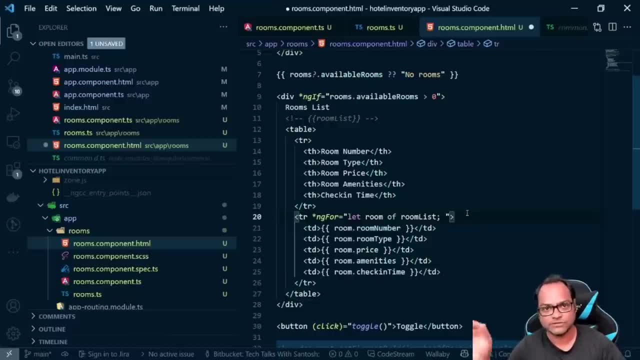 So in case I want to find out which row is even and which row is odd, ng-for gives you that. So I can say: let p equals to even and let o equals to odd, and let's print it here, right? 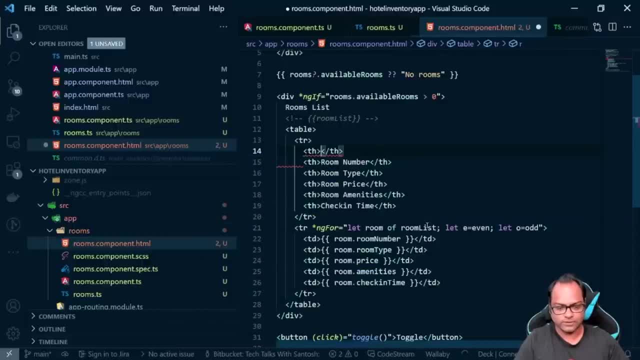 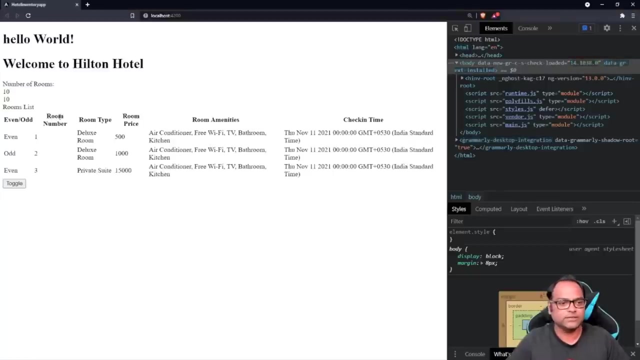 So I'll say: this is one more header, Even Slash, Odd, And let's see. So we're saying if it's even display even or display odd, Simple logic, right, So you can see: even, odd, even. 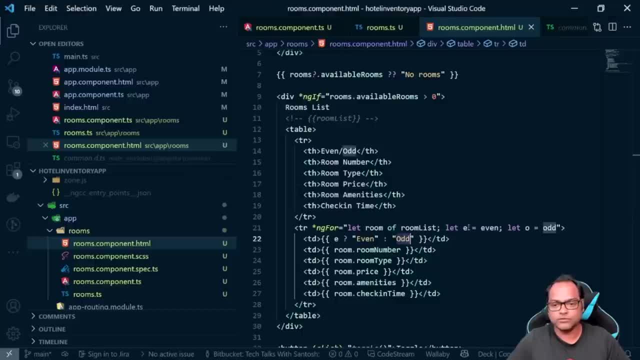 So this is how your information is getting displayed. So using even and odd values. What else? We also have an index value available, So, in case you want to get hold of a unique value for your row and you don't have any, 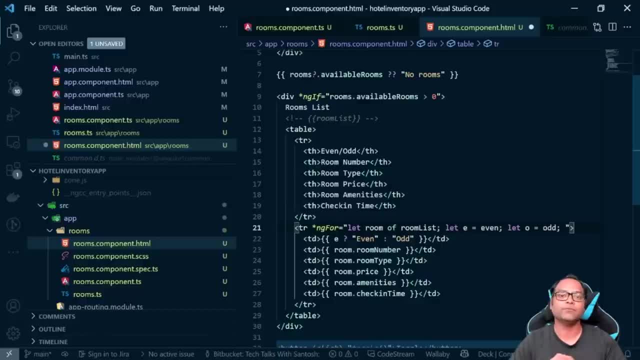 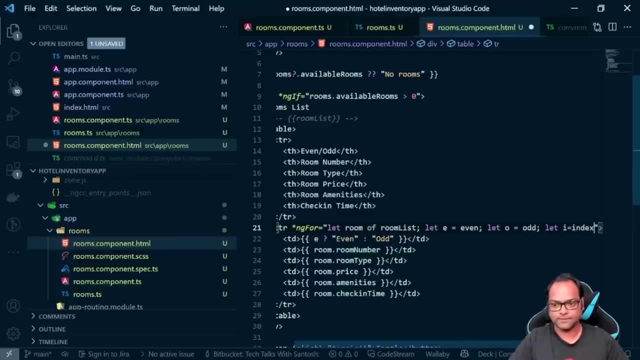 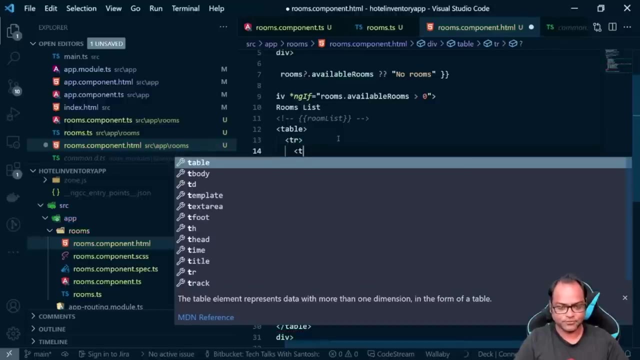 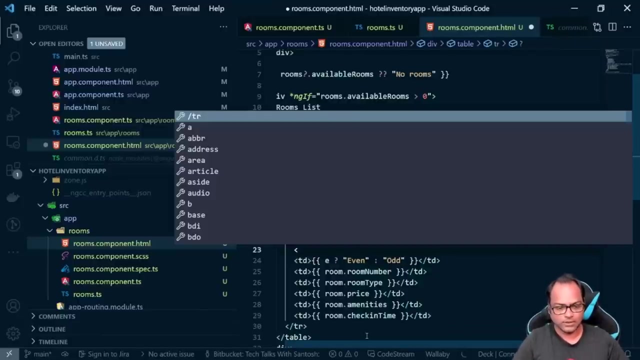 unique values. you just want to display a running number while actually displaying your records. That's possible. You can say let i equals to index, And here let's say I will add one more dh, And we can say dd, And let's say display i. 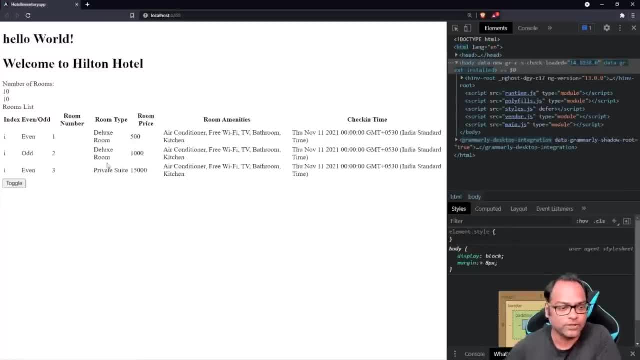 Remember, this is an index value, So it starts from zero. So don't be shocked when you see: okay, it's why it is giving zero because, of course, this is an index, So it starts from zero. 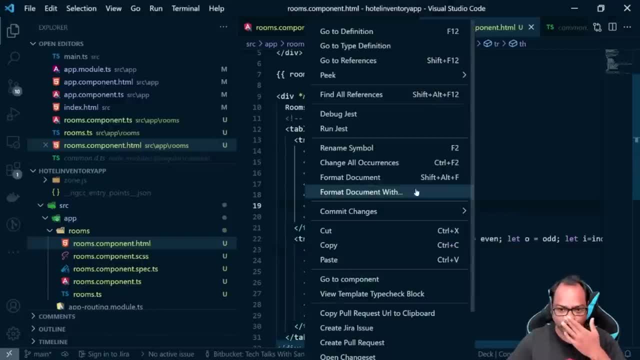 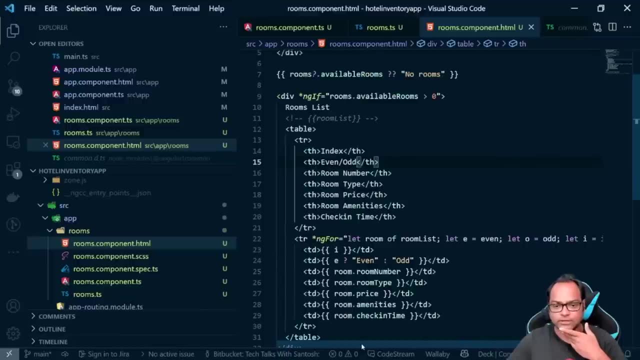 You will say zero, One, two. So this is it. So you have this few values which is available. We will talk about One more very important property of ng-for. let's do it later, because that will require. 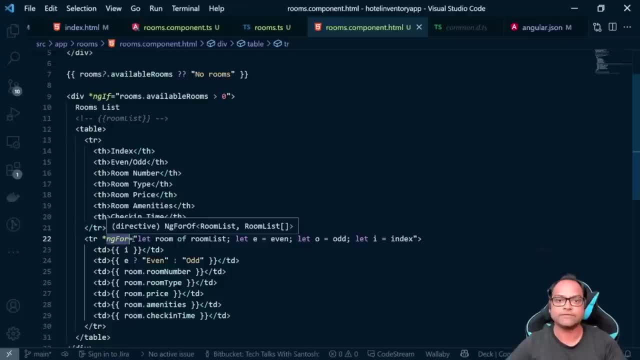 some extra code to be written, like we need services and all. to see an example: ng-for every time. the thing is, whenever you have ng-for directive used, in case something gets changed, it will re-render all the records within this data. 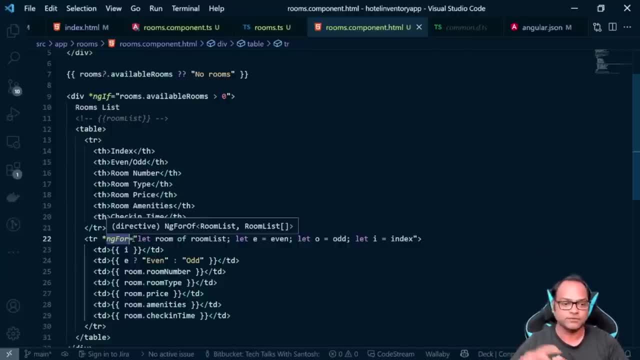 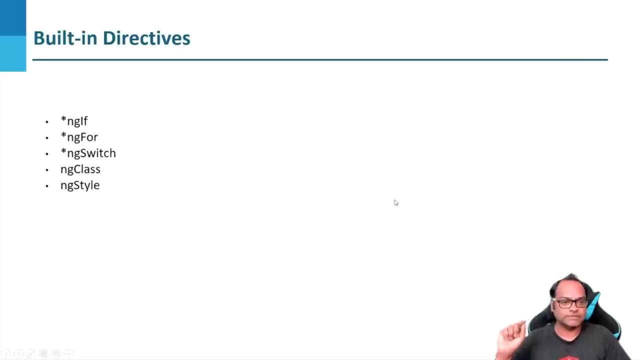 You can actually improve the performance of ng-for, Which we will see in a separate section how you can improve that- But right now, this is it. This is the basics which you need to know about while working with ng-for. So we are done with ng-if and we are done with ng-for. 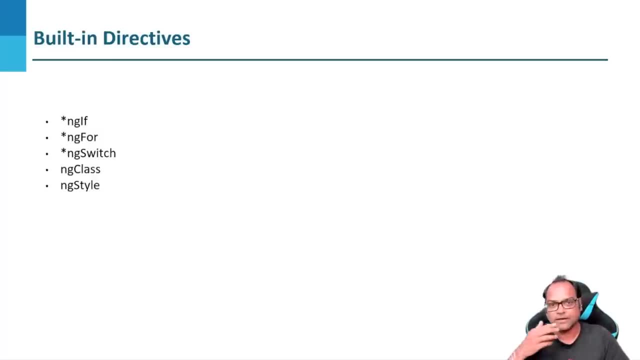 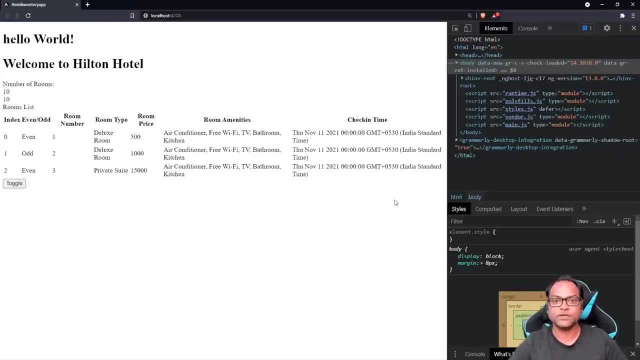 But we didn't discuss about one thing. You remember this star. What with this star is? Okay, we have been discussed about it, So let's talk about it. Okay, Let's talk about that star. Remember, we said there are two types of directives: attribute-based directive and structural directives. 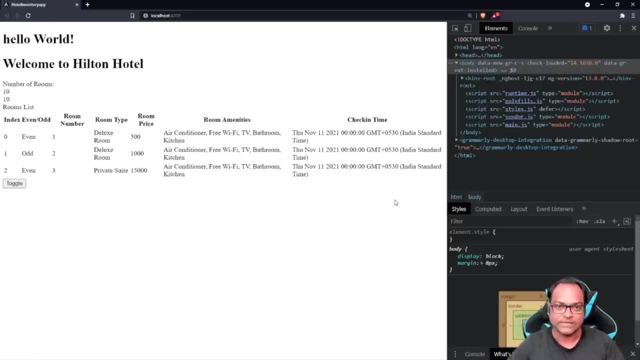 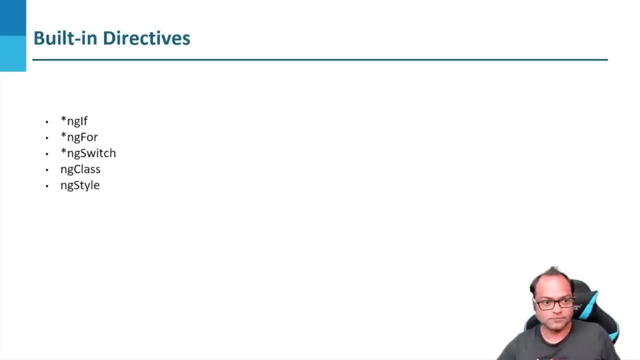 So how you will differentiate between structural directives and attribute-based directive. So that's the star which actually lets you know. or there is one more way: Generally, in all the built-in directives, which has star or structural directives? yes, that's true. 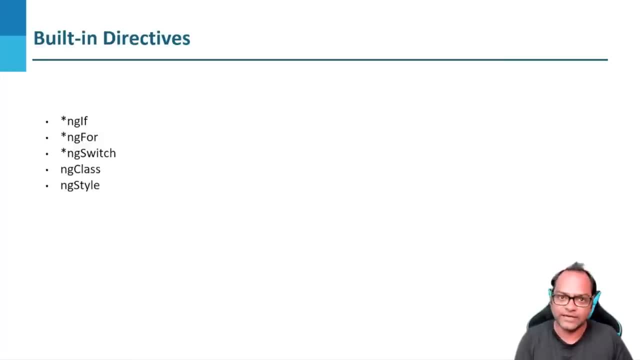 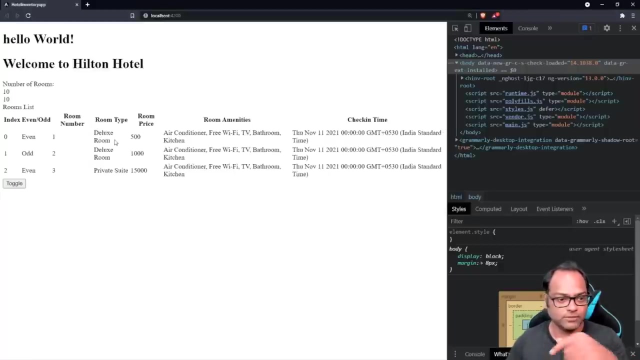 And other like ng-class and ng-style. they are attribute-based directive. So your structural directives, Okay, Okay, Structural directives can modify your DOM. Remember this Here. if you see your list on your view right now, you can see actually we just in our code. 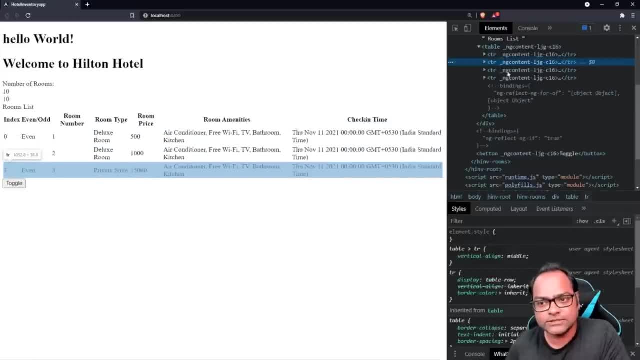 base, we just have tr-only ones. Who is creating this? three trs or four trs? one, two, three, four. Okay, First one is either, anyways. So one, two, three, Three records, right? Who is creating that? 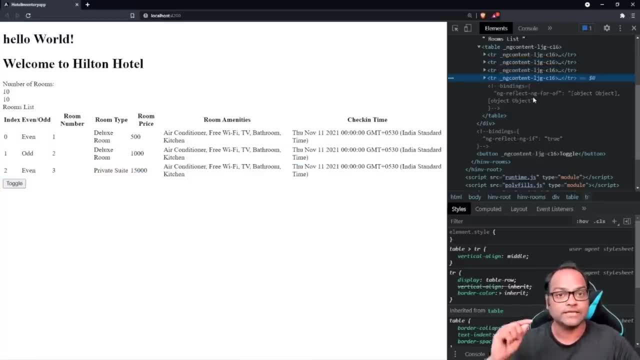 So that's the task of ng-for, Star ng-for, And it is actually a structural directive, so it can add or remove the DOM element from your view. Similarly, if you see, I mean we had used ng-if. it was actually adding the div or removing. 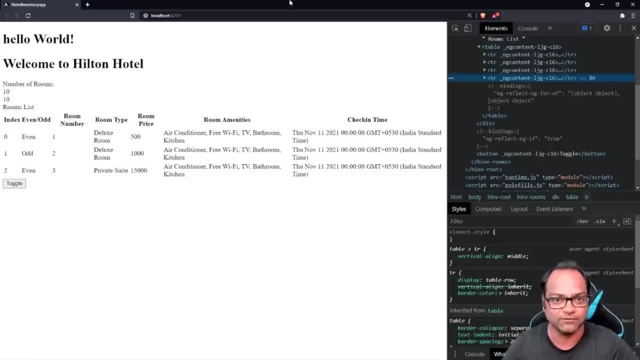 the div. You can actually do that on button click as well, of course, by changing the properties, So that also does the same thing. ng-if is also able to add or modify the DOM element, So any directive which can modify your DOM element is structural directive. 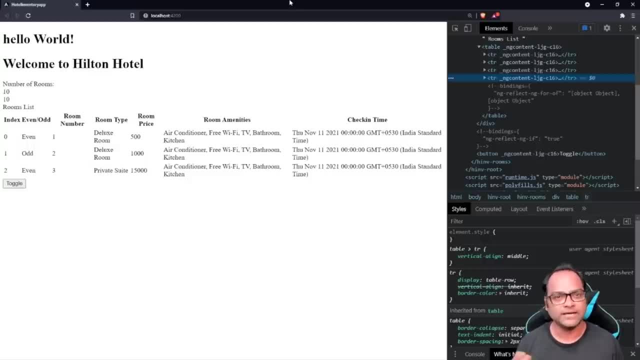 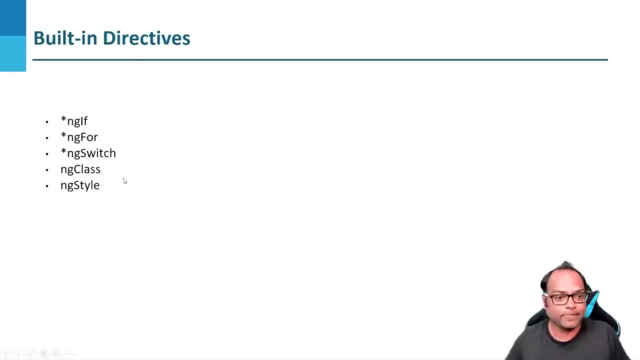 Attribute-based directives are something which will probably add some attribute to your element or remove something or add some extra logic to your element based on some properties, But they cannot modify entire DOM. that's the difference, So sorry. they can modify the DOM. 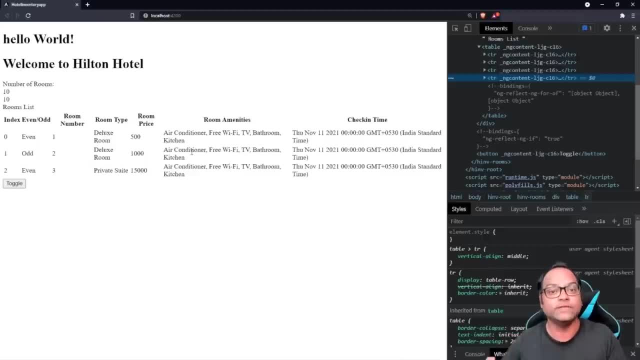 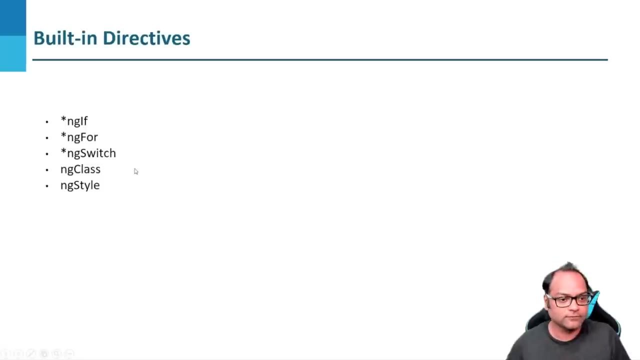 Let's, They can modify the DOM, But they can not add or remove the element from the DOM. That's what your attribute directives does most of the time. So let's see, let's talk about ng-switch. we'll take an example of ng-switch and then 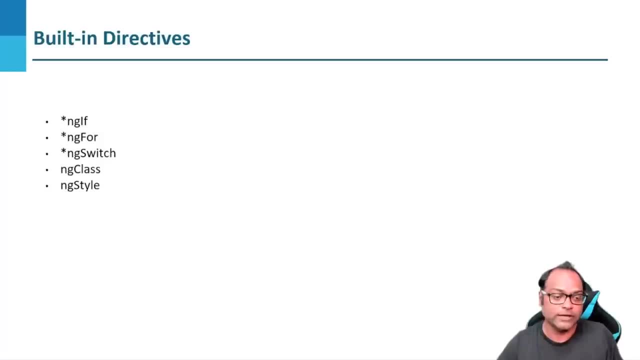 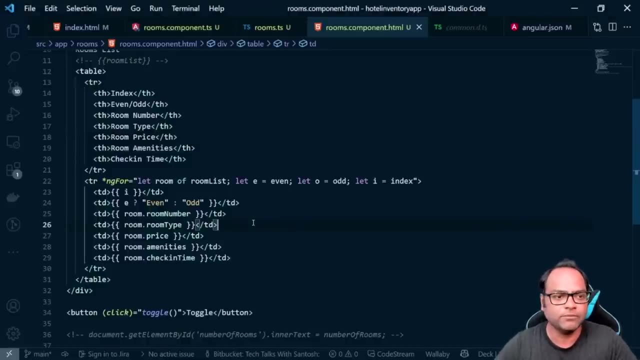 we'll talk about the rest of two class, two attribute-based directives which we have. ng-switch is something which is I have used ng-for. It's very, very rarely, but very useful. So let's see an example what we can do. 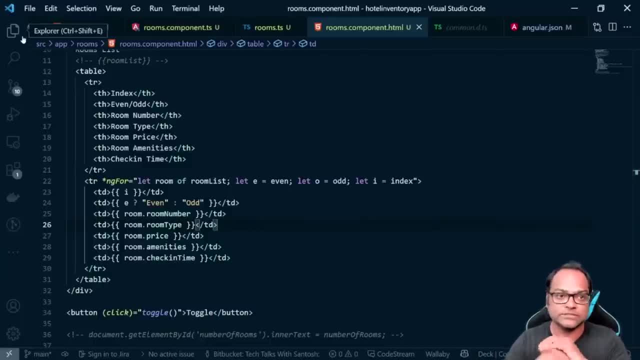 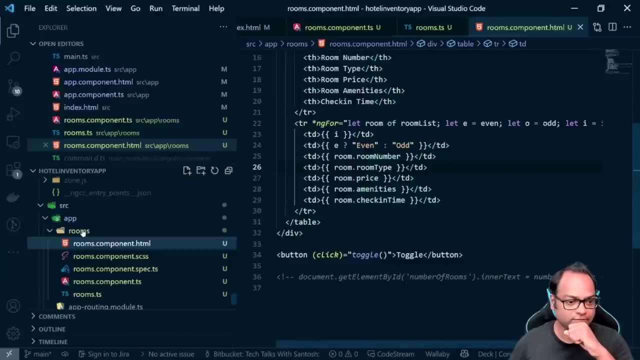 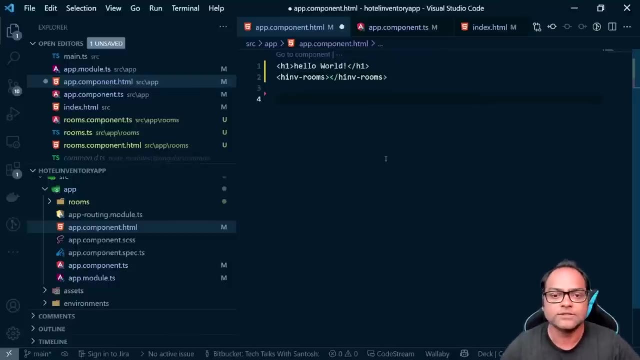 I'm sure you might have learned about switch case statement. So ng-switch is kind of similar, which is available here. So let's see what we can achieve. I'll take an example, simple example, here and let's see. So here what we want to do is, for example, if I am an user, I'm normal user, I don't. 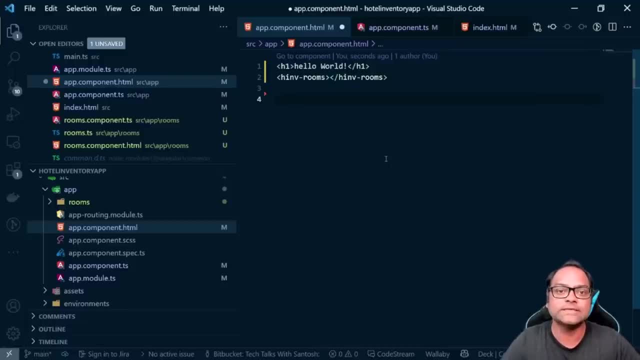 want to display this room's information to To the user. But in case I'm an admin, I want to display this rooms. So let's see how we can achieve that using ng-switch. So first, what we will do is we'll create a property here. 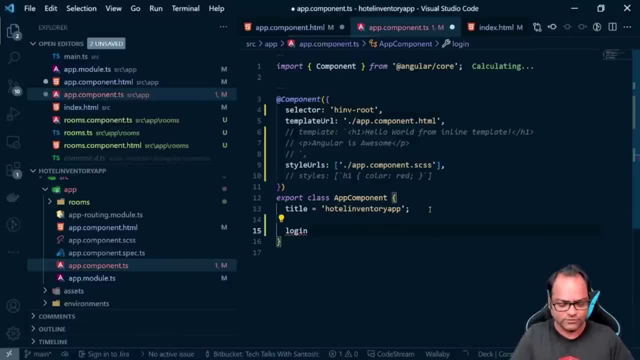 I'll say this is login type. We don't have login page right now, so we'll just start with mock data. I'll say login type and I'll say this is admin right now And let's go to app component or test statement here. 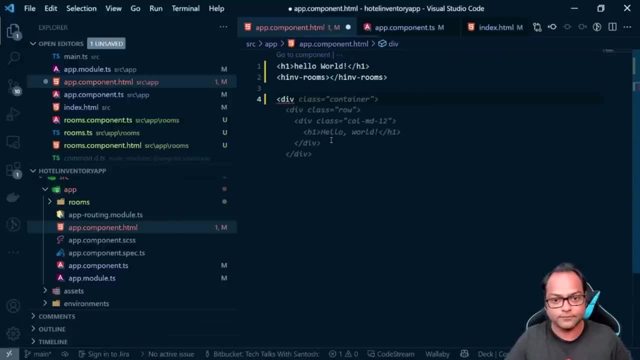 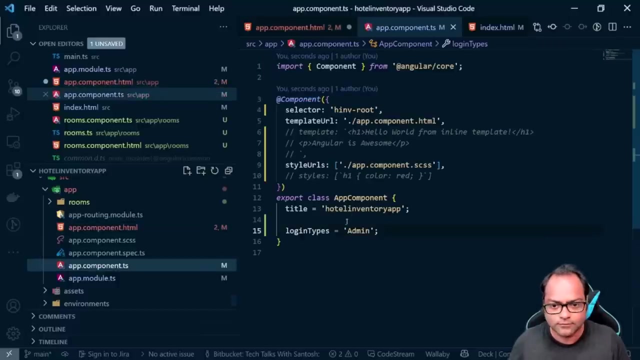 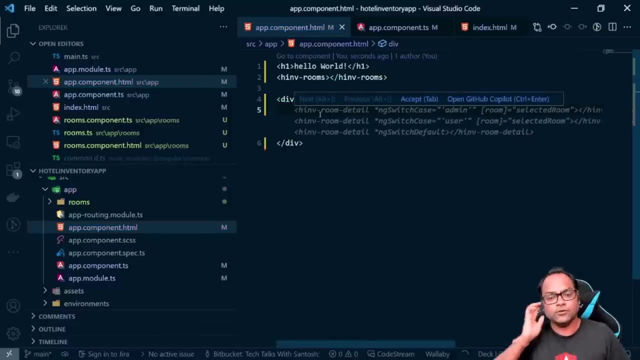 I'll use a div And I'll use star. ng-switch is equals to. I'll say: this is login type. just a second. Or let's name it role drive, which makes more sense. Okay, And now, based on whether the role is admin or if it's simple user, we want to display 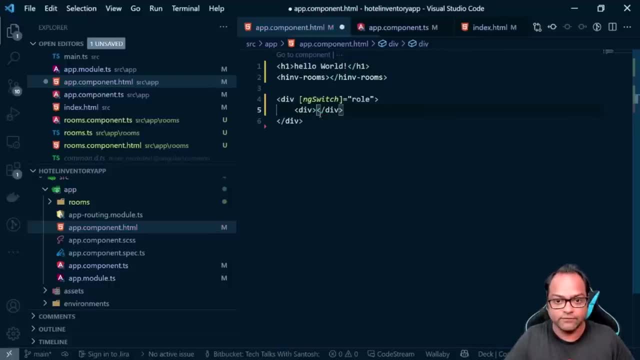 different views. So here what I will do is I will say a div and we will use star. ng-switch case is equals to. I'll say: this is user, This is user role. I want to display, I want to use it as string. 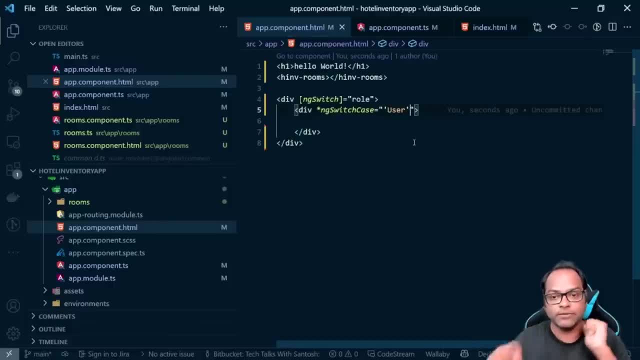 So what I can do is I can put single quotes inside it. Remember, if I just remove single quotes, it will treat it as variable, as we have seen so far while binding the data. So here I want to treat it as string. 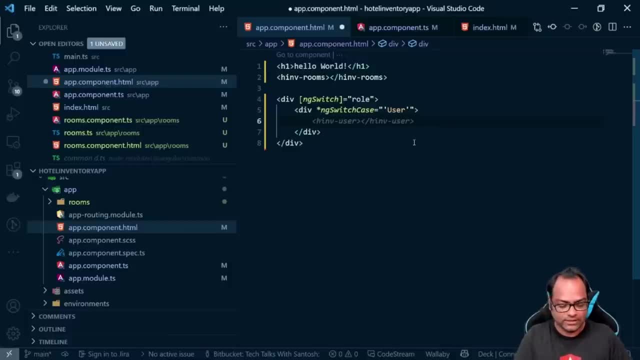 So I'll say, okay, this is a user, And here I can say this is, let's say, welcome user, right? So this is what you want to display to the user. If it's not, it's admin. 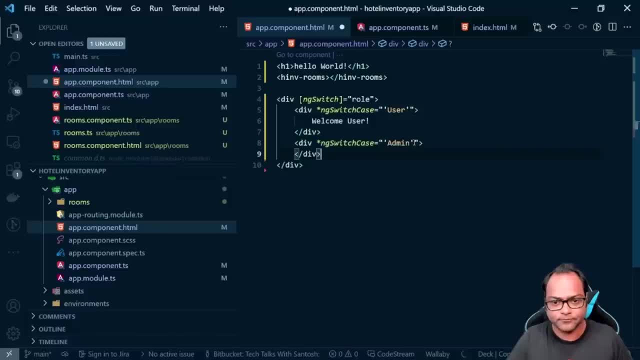 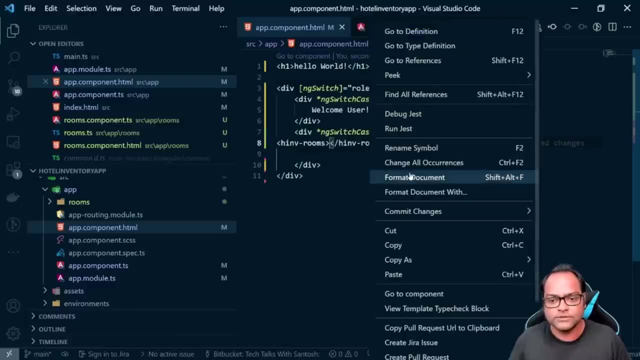 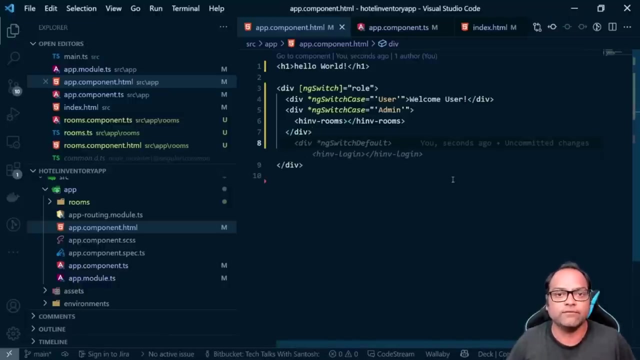 Okay, I want to display this rooms information and a switch case like a switch case statement. This also has ng-switch case will also have a default one, So you can use that. So default, I can say you don't. 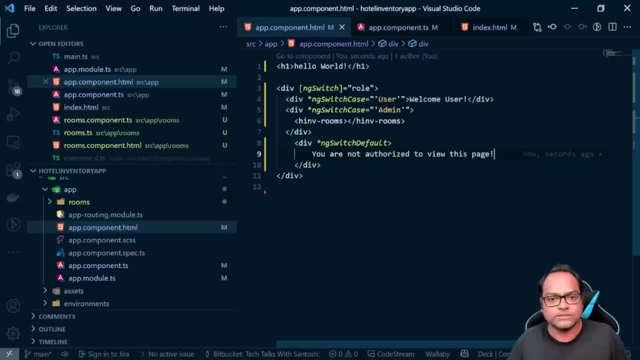 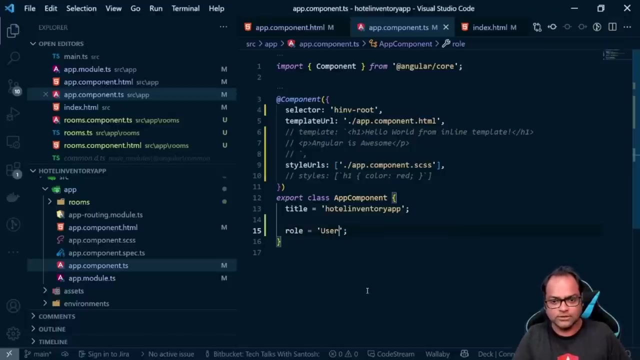 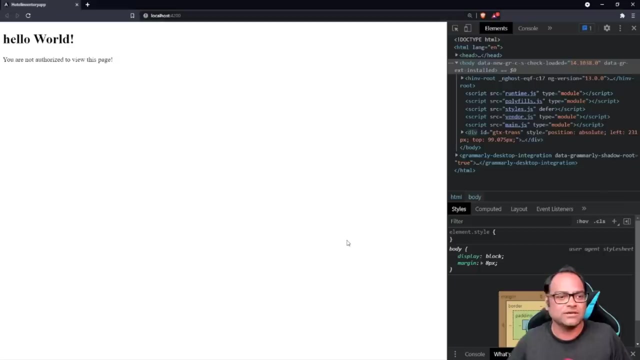 Okay, You're not authorized to view this page, right? So let's see, right now our role is admin, So we should be able to see everything. Let's change our role to user, So we'll see that welcome user thing. So you can now have welcome user and let's type users, which will say you are not authorized. 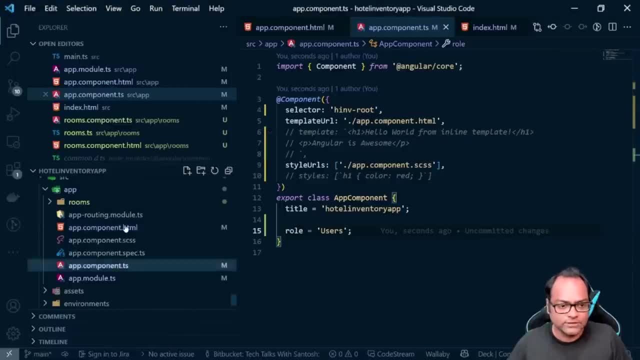 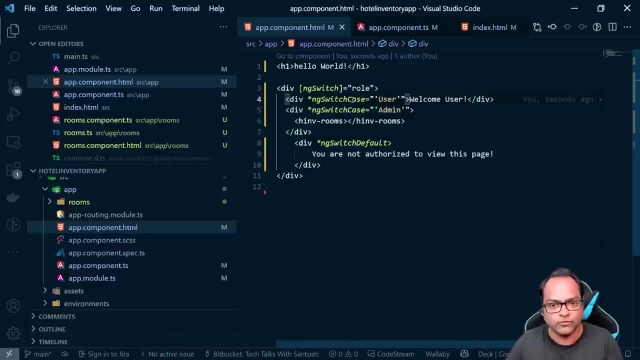 to view this page. So this is your ng-switch case works. So you have like your ng-switch, So where you are assigning the value, and then ng-switch case based on which you can toggle your view. You can display whatever you want to here. 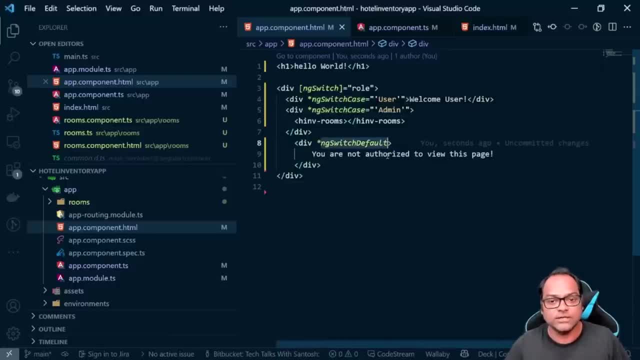 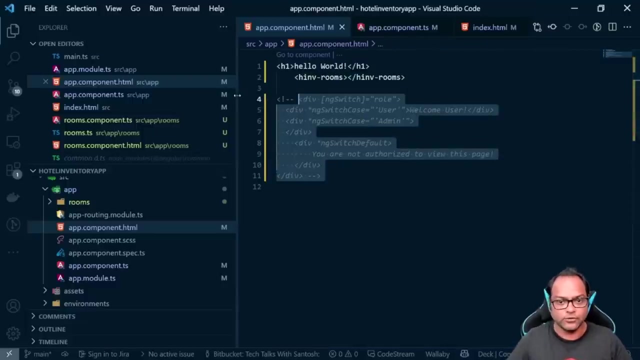 So ng-switch case and ng-switch case default. These are the different attributes- or you can say different directives, which you have available. You can use those. We'll keep this code here because we are not going to use it anymore. So Okay. 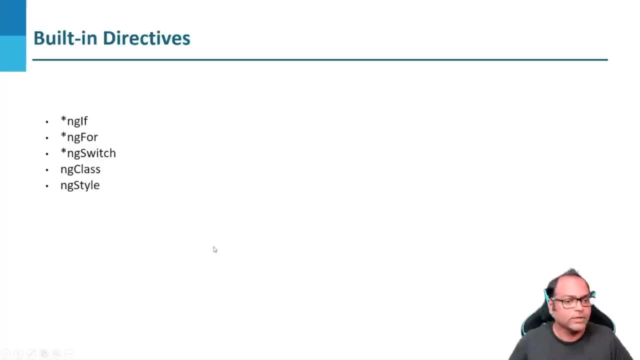 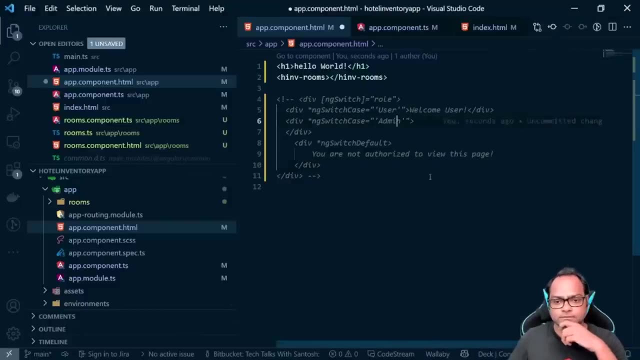 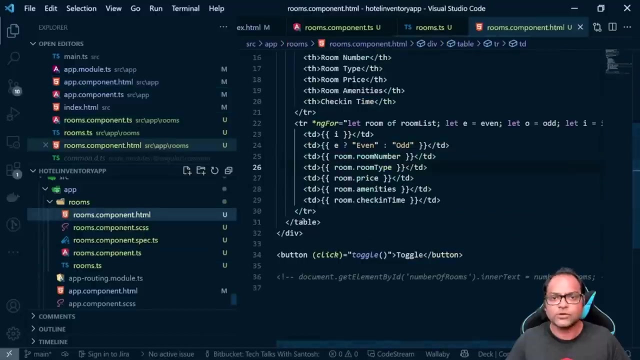 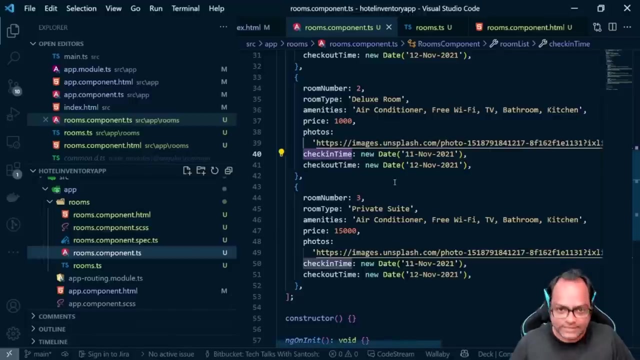 Let's see an example of ng-class and ng-style, and then we'll wrap up with built-in directives. So can you guess what ng-class and ng-style is related to? Yeah, If you. if your answer is related to styles, yes, that's, that's the correct answer. 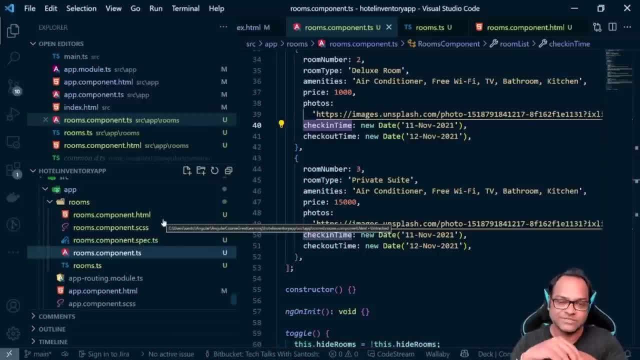 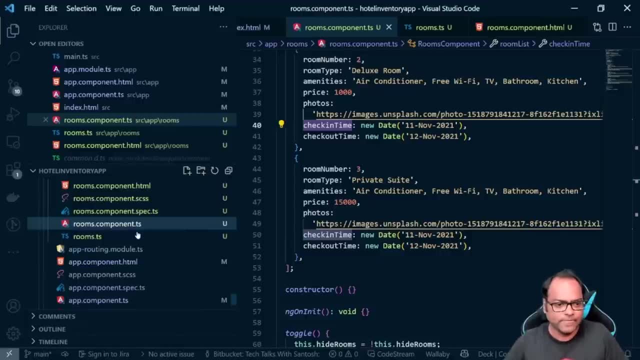 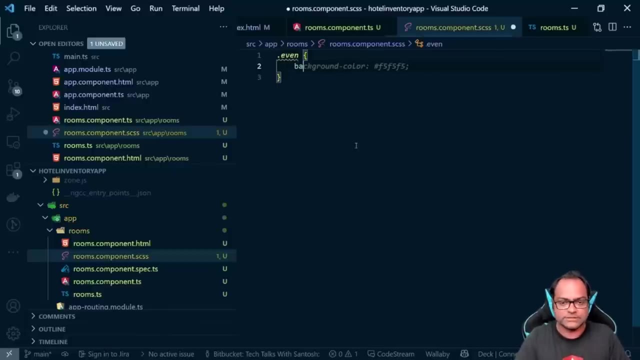 So what we need is there are two ways right, So I can just upload it, So I can just apply some style, or I can apply some some class directly. So let's see how we can do that. So here I'll create two classes, even where we have, let's say, background color and color. 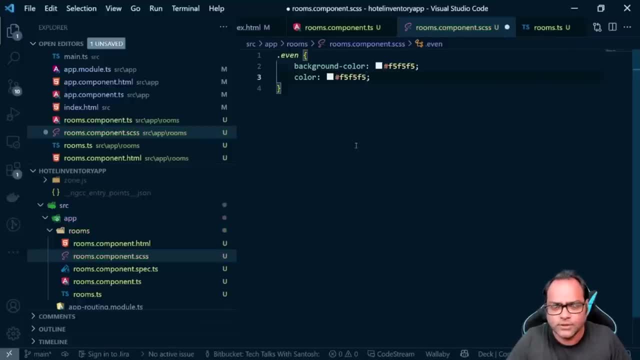 Let's change to. this is looks white, So I'll say: this is still blue And let's change it. And color is white. And then there is an odd class which has background color of light steel blue And let's use tomato and white. 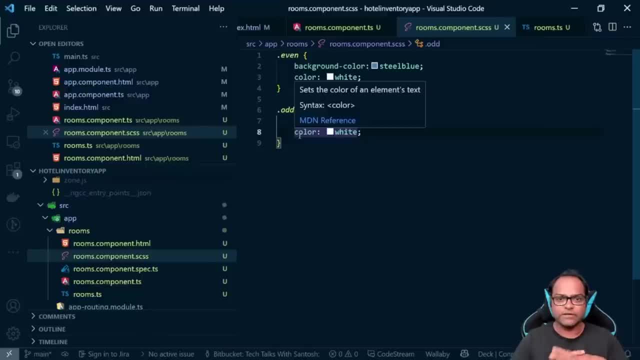 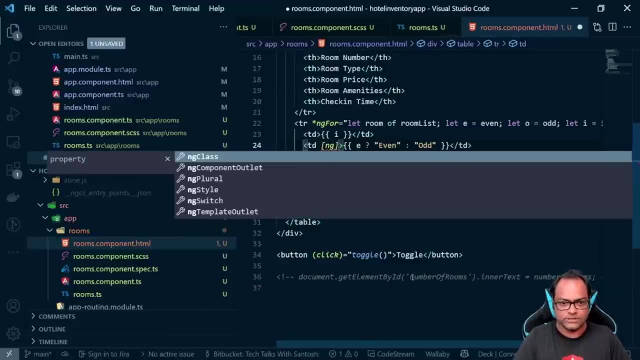 So let's see how you can use ng-class to toggle the class between even and odd. We can do that here. So I can apply this ng, not here. Let's see, I can do that. Okay, So let's not apply on td, we want to apply it on tf. 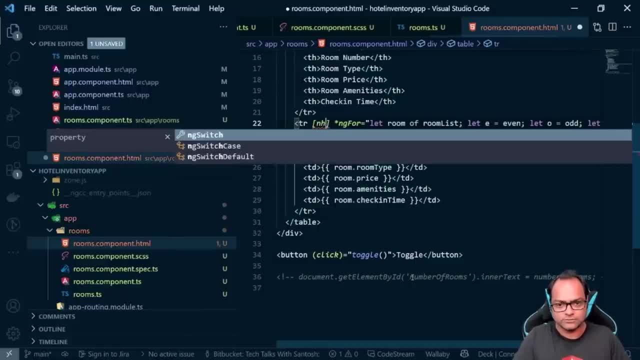 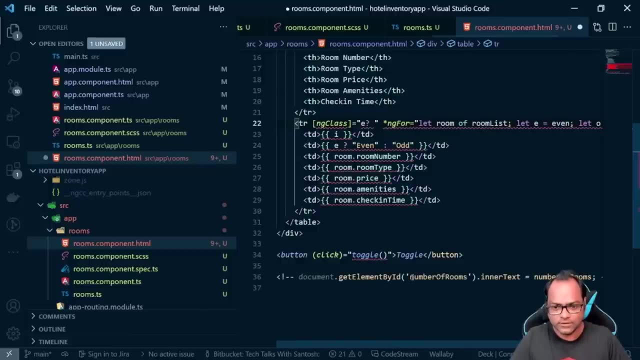 So I can say ng-class is equals to. so if I'm, if my class is even, then I can say: okay, the, if it's even row, I mean my class will be even. else I'll say: use odd class. 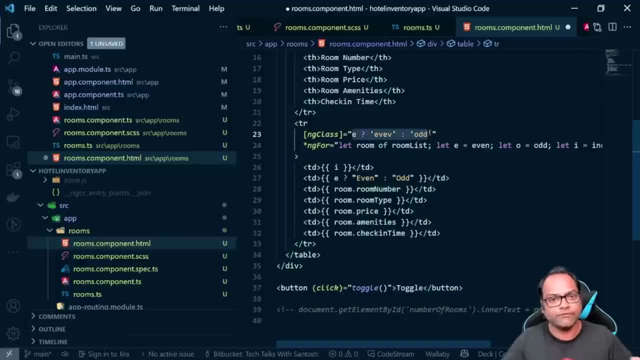 There are multiple syntax, Remember. you can also just use a variable name. I'm directly here. That's absolutely fine. Right now we are saying, okay, based on even value switch, have different class. let's change this to even. 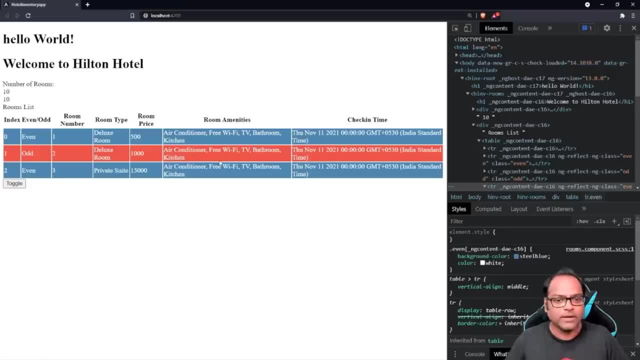 Let's go to view And you can see we have different rows, different background color for different, different even and odd rows, Right, So this is how you can use ng-class. Also, as discussed, you can also have a variable. for example, let's say you have a class name. 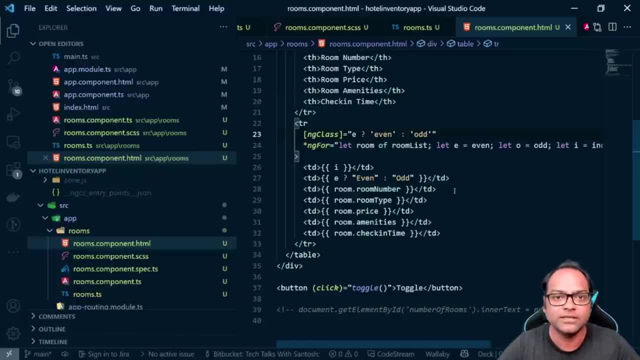 which is saved for some user, user preference: Okay, This is right, They they prefer some different class to be used, So you can save those, those class, and then load it via variable. That's also possible, And this style is something where you have to give the style. 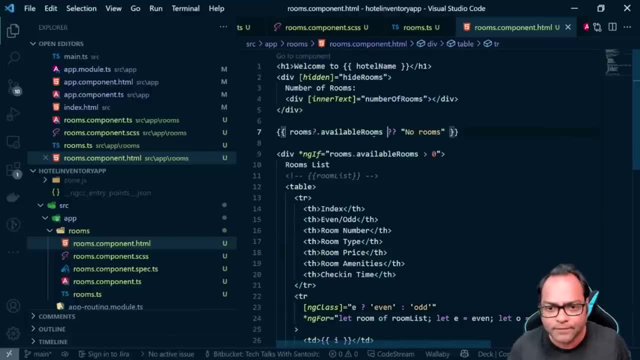 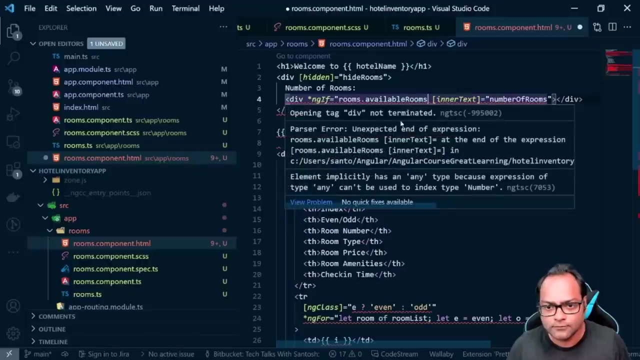 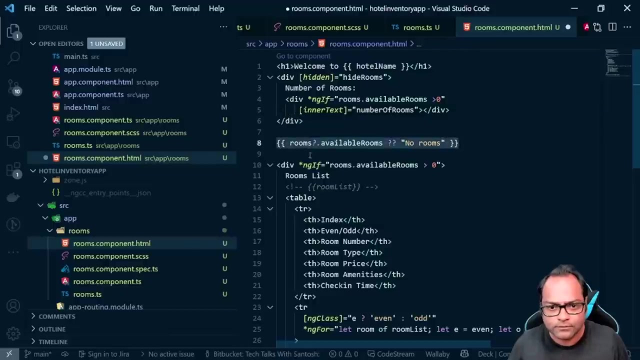 So let's see where I, where we can do that in a text here. let's try to do here. So I'll say if ng ng-if. I'll say ng style, I'll say ng style. no, I'll say ng style. no, not my style. 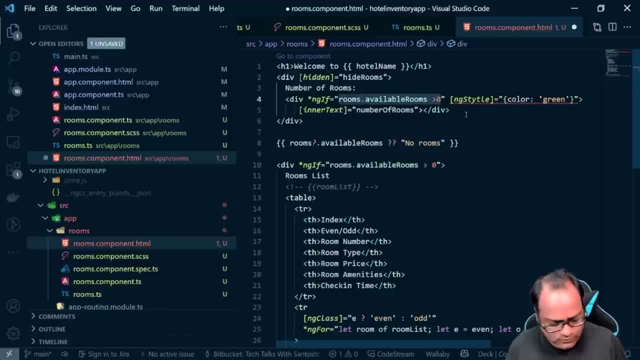 rooms. let's remove it right. i mean, we can directly do this as well, so we can say here rooms greater than zero, room style available greater than zero. then we can say color, then color is green. so we'll just see this one. let's see if this works, because i generally 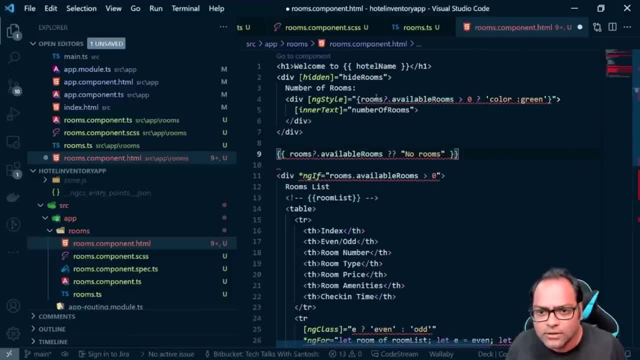 don't use ng style. okay, it is expecting something. at length, rooms are color green. uh, missing, expected curly brackets on line number seven. this is close. this is okay. okay, this is an extra right. oh, what a question, right, you can actually we can do something like this, so we can say color which is a property and then 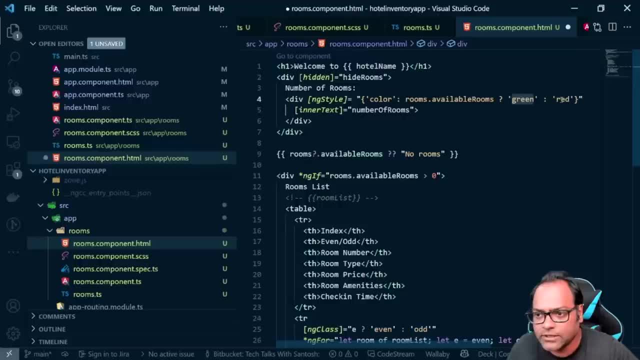 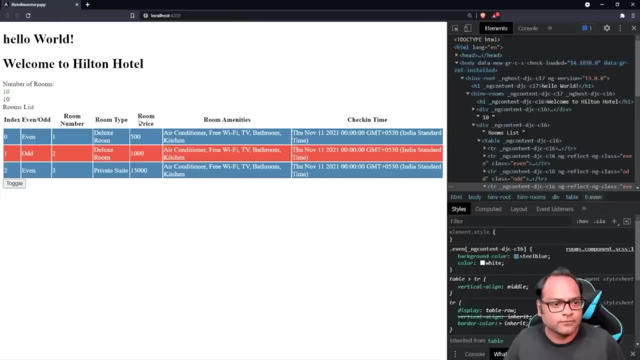 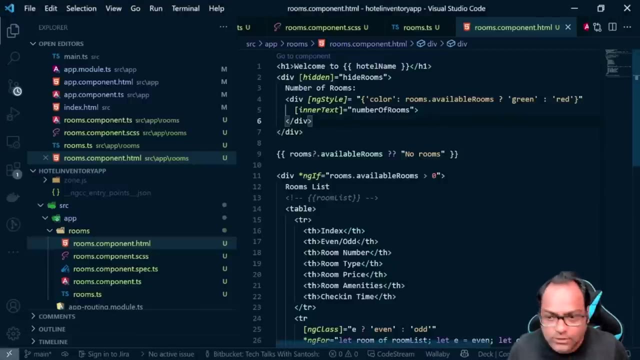 we are saying: if rooms, there are available rooms, make it green, otherwise make it red, red. let's see how it looks like. we can see this is green color which is coming here, so let's make it some other color which looks visible. so i'll say steel blue. 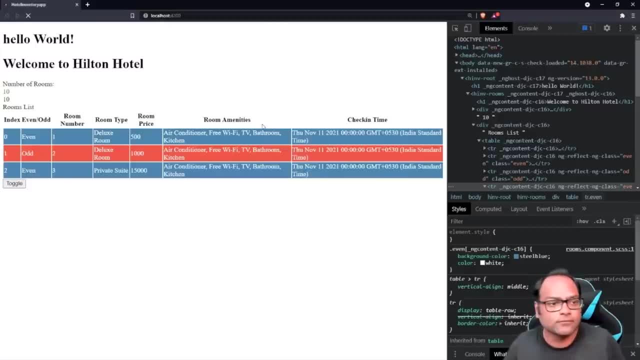 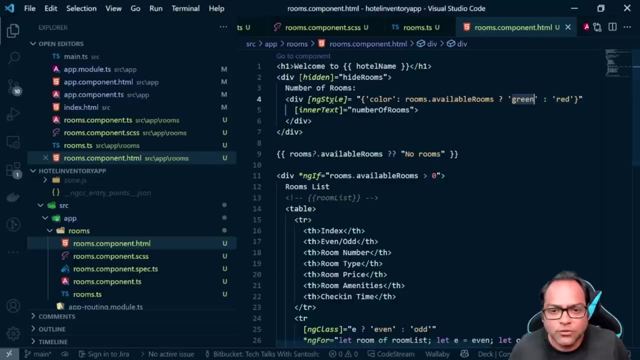 okay, so this is steel blue. now you can see, of course, that it is different from the the black, or you can just keep it green. so this is how you can also use ng style. ng style also accepts variable, so you can also pass a variable here, that's. 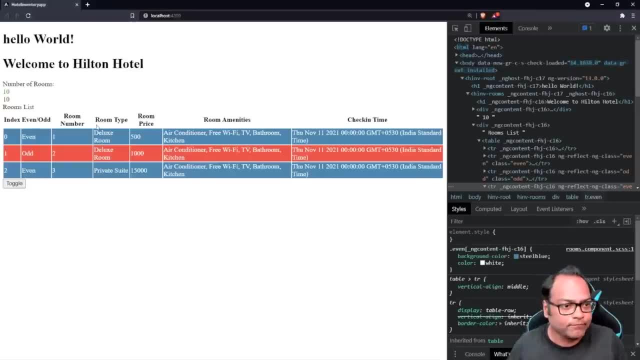 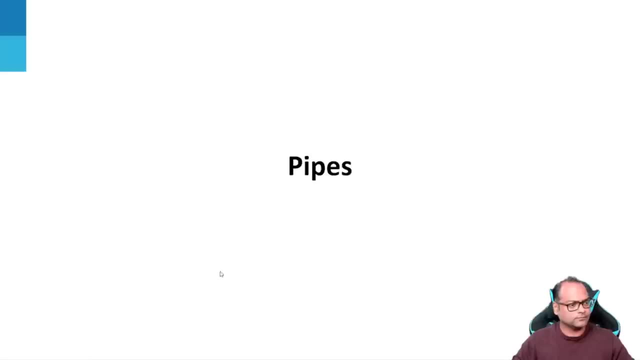 absolutely fine. so you can also pass a variable here. that's absolutely fine. so this is from the directives part. now we will move on to pipes. so we know how to do data binding. we also learn about a few useful directives. next thing which we are going to talk about is pipes. 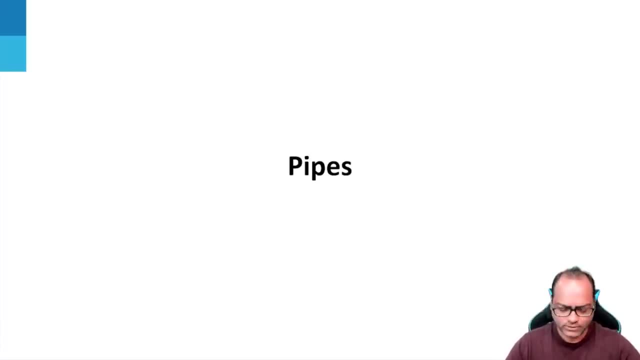 what is pipe so in uh. so we are going to see what is pipe and then we will talk about some built-in pipes. so let's first talk about what is pipe so in your day-to-day uh work. of course, what you will be doing is you will be binding some data on your uh front end screen, or your view, and there will be times. 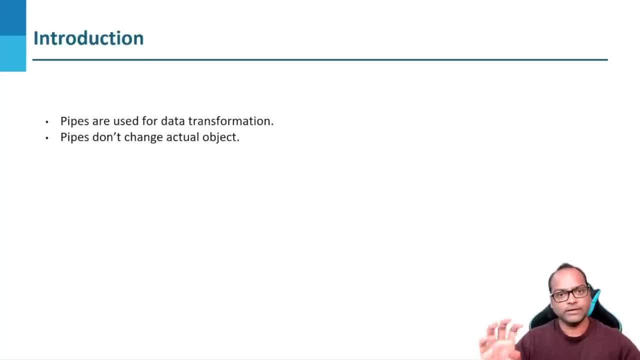 that a requirement may come that, okay, this particular date object should not be displayed in the long date format which we have seen. probably it needs to be shown in some other day format. or there might be requirement to display amount in, let's say, dollars, inr or any other uh currency, right? so by default the currency is: 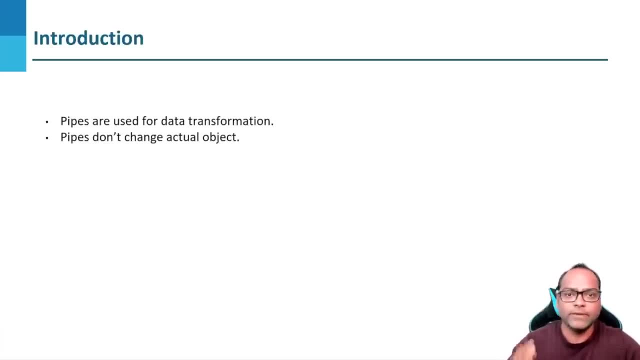 uh, dollar, of course, but we may need to actually show it in a different format for it's uh. the same goes to numbers. what to do? i mean, of course, we cannot ask the api to change the date format. they will be like: okay, this same api is getting used at multiple places. so what we need to do is we need to. 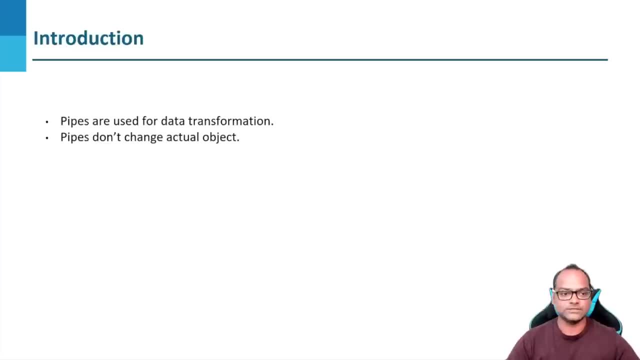 change the date format. so how do i know when the pipe is right? how do i get data in order to tell me? why should i do that for you? so the pipes are the answer. so pipes are used for data transformation. so when i mean transformation, it has a meaning. so transformation means my original object remain as it is. i'm not going to. 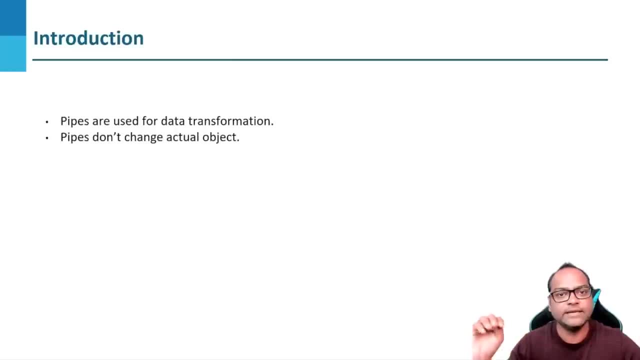 change that object, but while presenting that object i am displaying it in a different format. so it means the pipes don't actually- uh, pipes actually don't change the usual object, they keep it as it is. but while your view, you may actually change, deform it in different, different formula. so there are few. 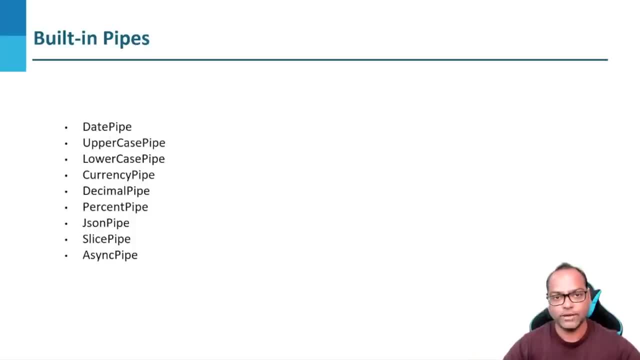 built-in pipes which we have, and there are few. uh, you can actually write your own pipelines, which we are going to do in future. here we will go through all the built-in pipes which we have. so you, we have dead pipe, uppercase, lowercase, we have currency, we have decimal, we have percent pipe as. 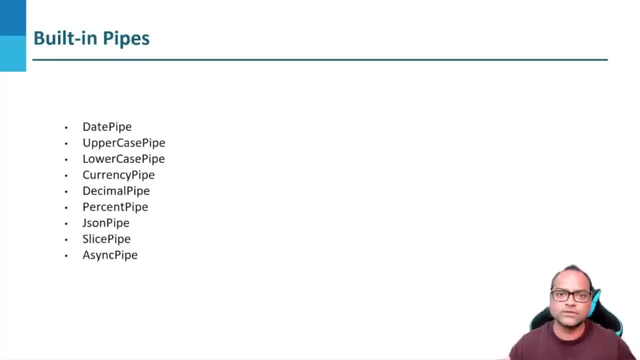 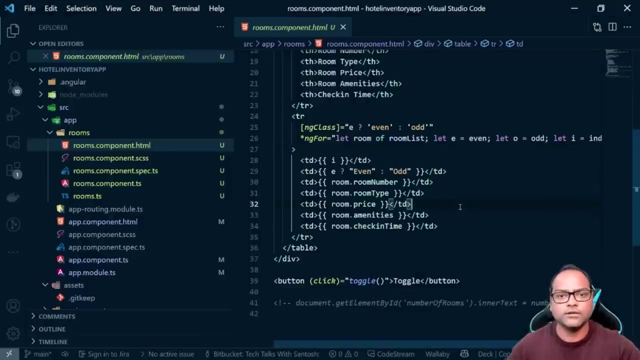 well, we have json pipe slice and then we have a single. so let's go through them. uh, go, go. so let's go through them one by one and we will see. uh, we will apply and then see how your view looks like. so let's switch back to the vs code. and this is the same view which we uh wrote last time. 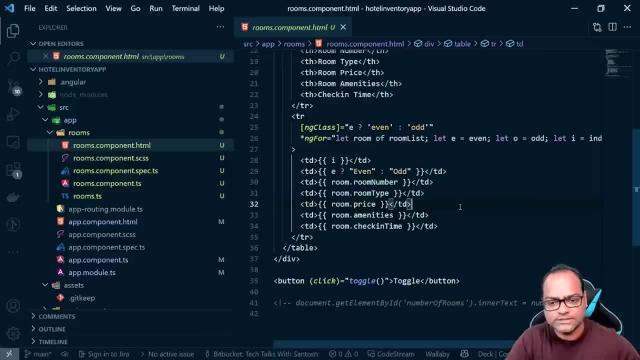 so remember rooms, and then we created a list. so let's start with the first pipe which we have, which is date pipe. so we already have a property called uh check-in time, right. so here let's uh see how we can apply pipe so you can give uh use this particular symbol. 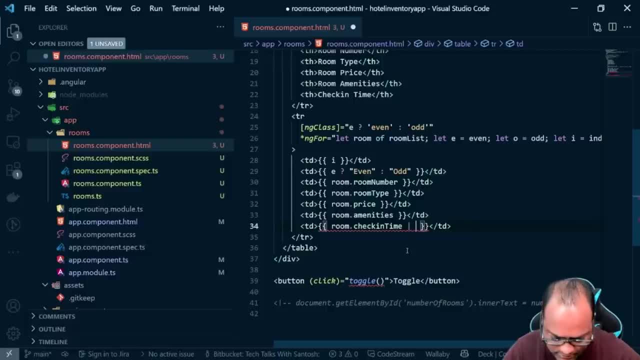 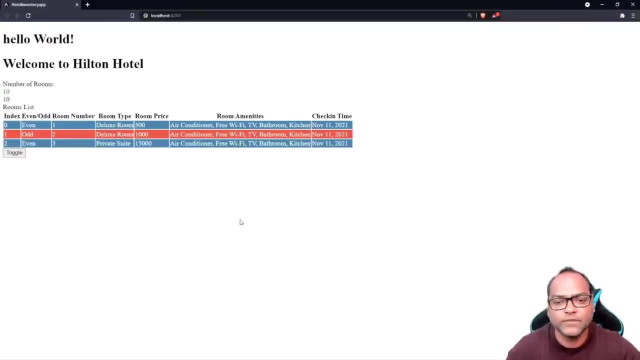 which is available just below backspace and above enter, so you can just shift and press this, which is pipe operator, and then you can write: okay, i want to use date pipe and let's go ahead and see this and, uh, let's see it on our view so you can see your date time format is actually changed to. 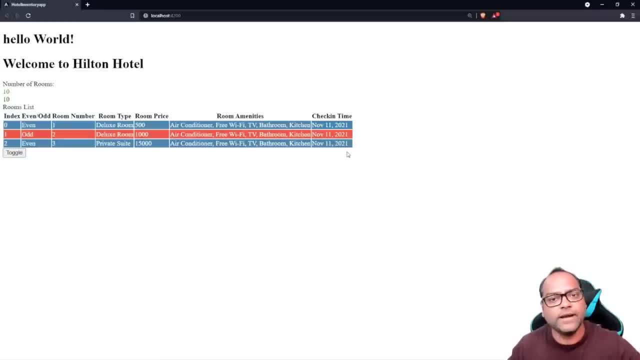 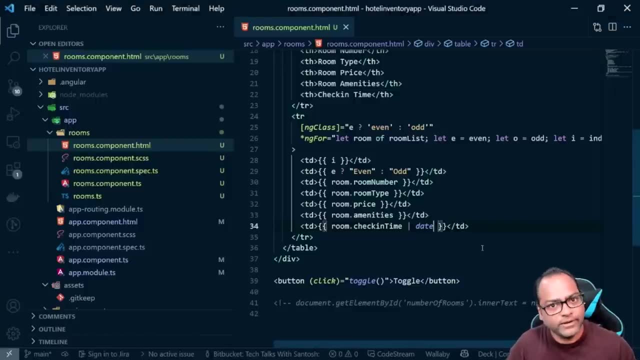 something else. earlier it was a long date format. now, once you apply date, it is short date format by default. you can also change it uh with specific date format. you can also change it uh with specific format as well. all the formats are available on angulario docs so you can just. 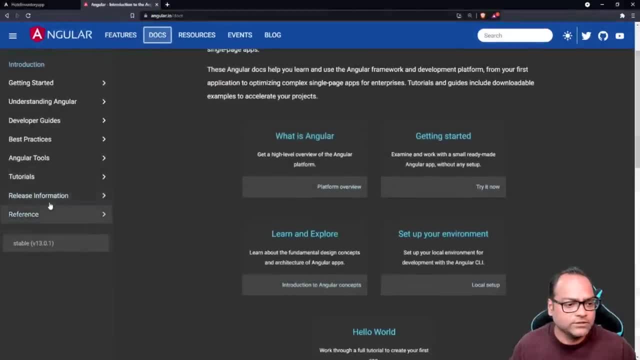 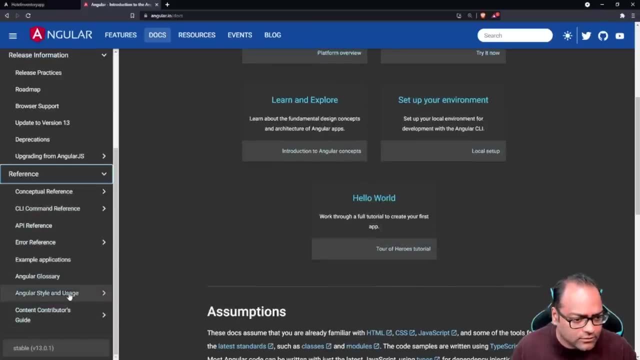 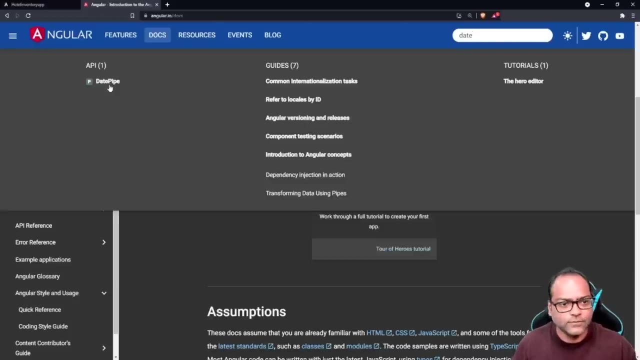 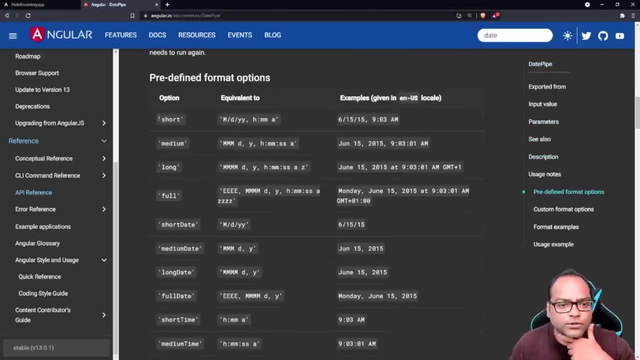 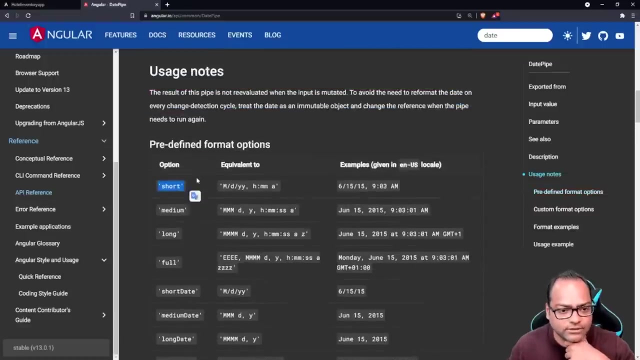 go to angulario and in doc section you will see uh references. okay, so it's under api. so you can see all the formats you can use here. so you can also use text short, medium, long, or you can also specify the format you want as well. so it's up to you. so let's say, if i just say date and then uh, in case, 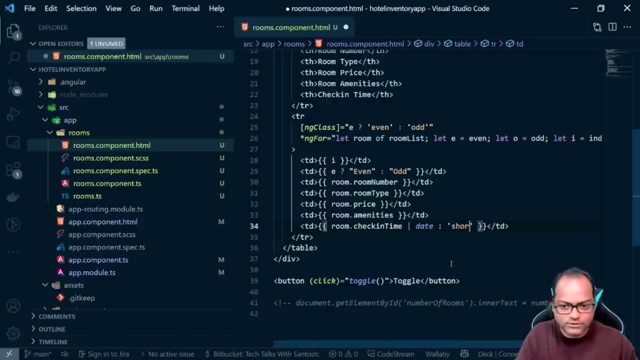 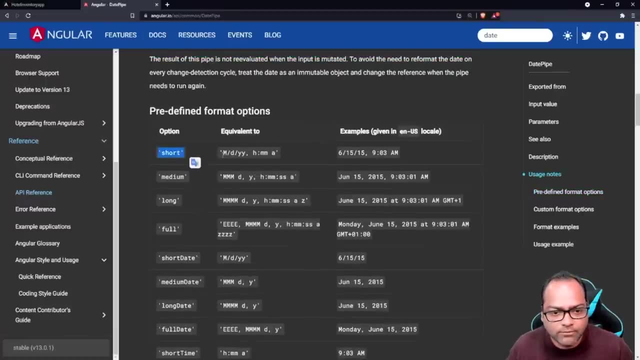 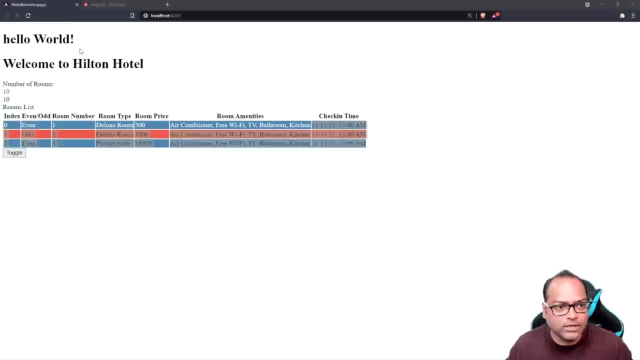 you want to change, you have to put colon and then you can write: okay, short. so this is the format which i need: short, which is the equivalent to, let's see, m, dd, by, by, h, m, m, e, so it's like the example, right? so, uh, the one which is by default, is this one short date you can specify. 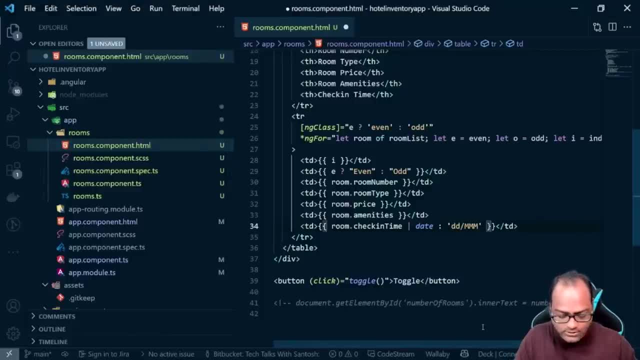 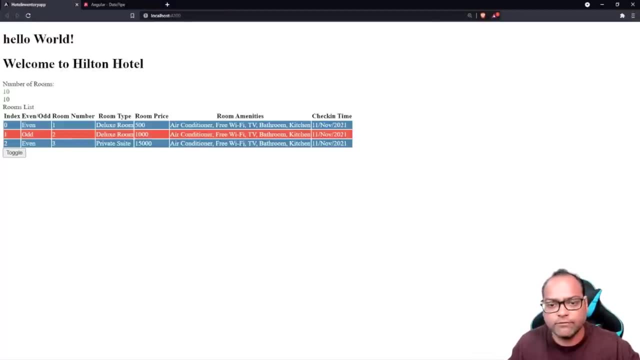 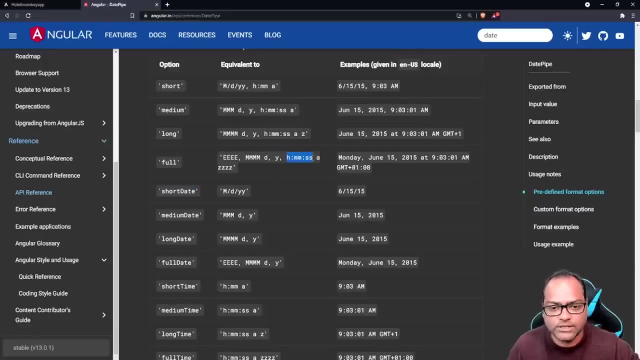 the format as well. so i can say dd, uh, mm and y, y, y, so it will be a date, month, in the first three characters, so you can say 11th november 2021. so this is how you can actually change the formats and you, in case you need time, uh, so you can also pass the h, m, m, s, s and uh, uh. this one, two, three. 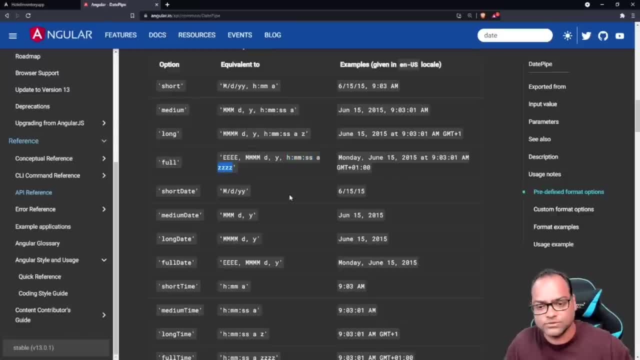 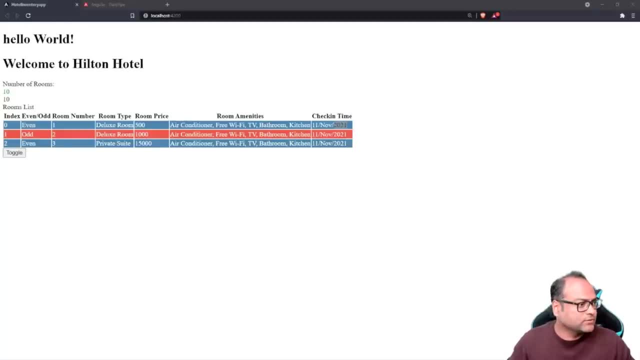 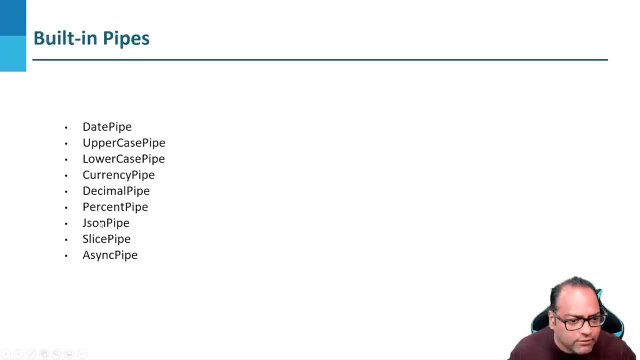 four. four sets is actually for time zone, in case you want to display the time zone. so this is an example of date format. let's see what else we have. so let's go back to the slides. we have a bad case, lowercase. let's see both. and then, um, we also have title case, okay, which i missed. 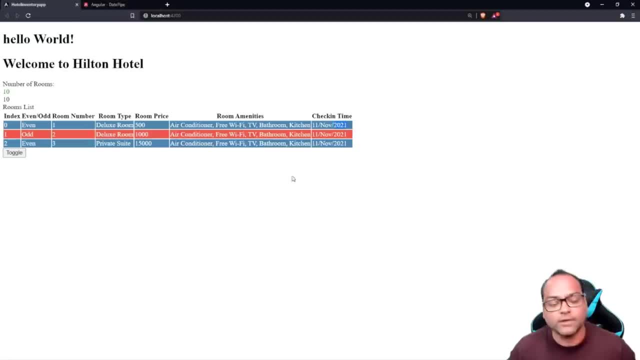 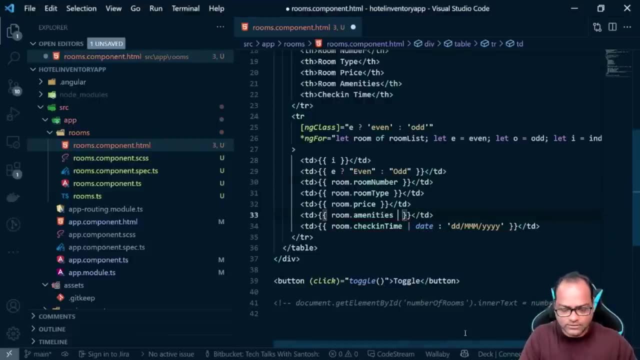 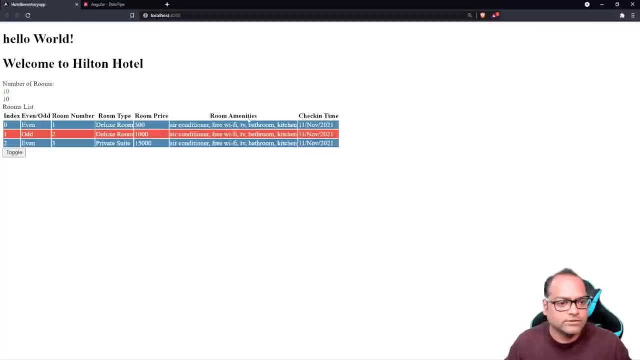 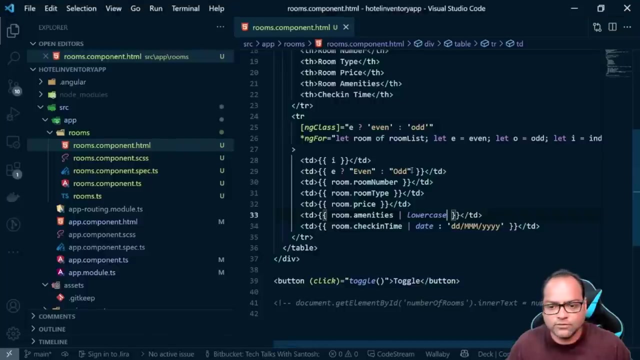 here to them, okay. so let's say, uh, amenities, right, so i want to display this in lowercase, so you can say lowercase, so everything will be displayed in lowercase characters and so you can see air conditioner, free wi-fi, tv, bathroom, kitchen, or everything is in lowercase right now and up, and i can just change this to uppercase and everything will be in caps and 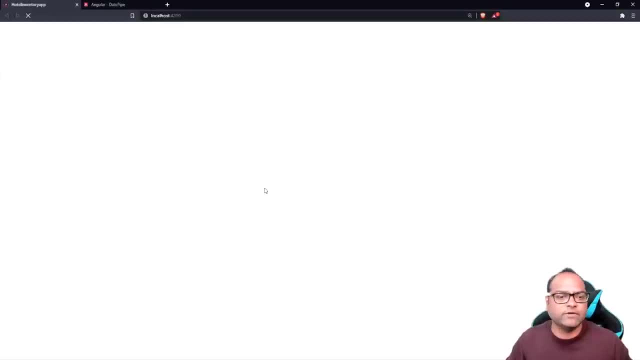 if i'm not wrong. okay, so i missed it in slide, but we do have title case as well, where the first character will be in capital. so you can see air conditioner, free f, and then we have tv, bathroom, kitchen, so every the first character is in capital. that's title case free. 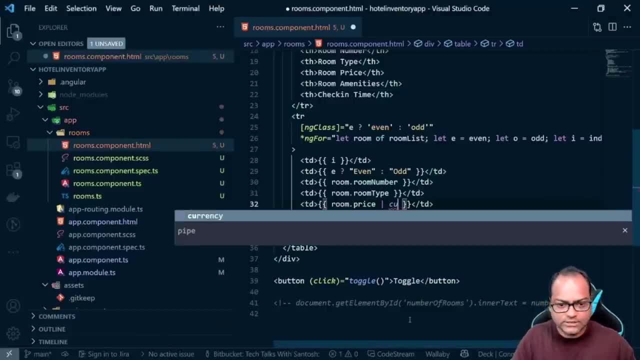 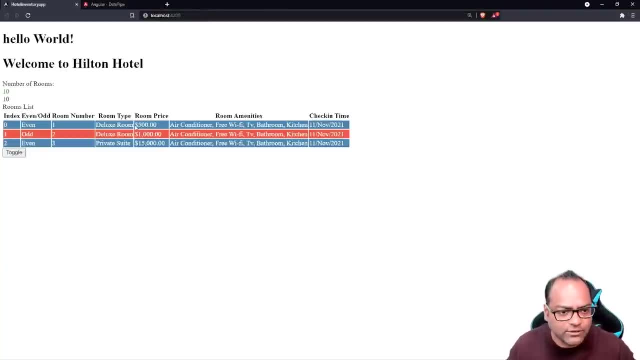 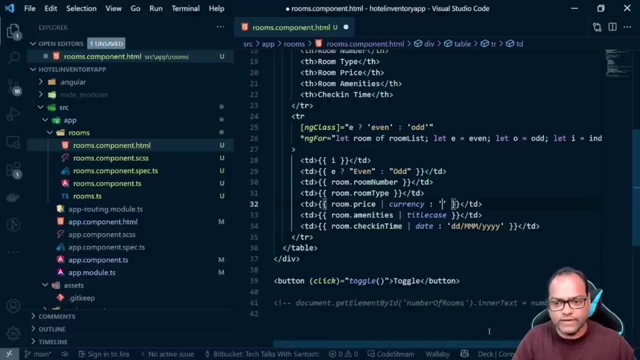 now we also have currency so we can use currency and, by default, the default currency is in is based on, i think, en us, which is dollars, so you can see dollars available here: five hundred dollars, thousand dollar and fifteen thousand dollars. you can change currently by passing the value, for example, uh for uh- indian currency. the co-designer. 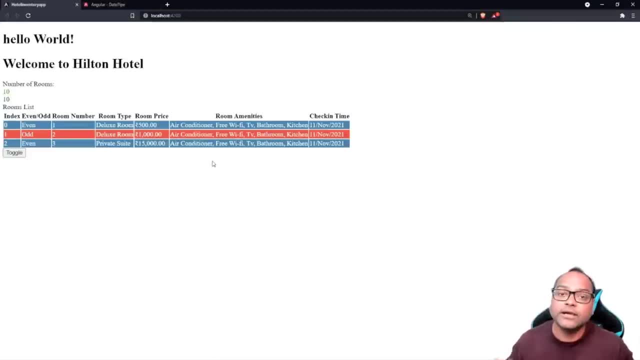 so you can see uh. it will now give us rainbow symbol. remember the currency uh code to its equivalent uh display. uh is not available for all the currency types. it is available for all the major currencies, but you may actually find some currency which is missing, so in that case, 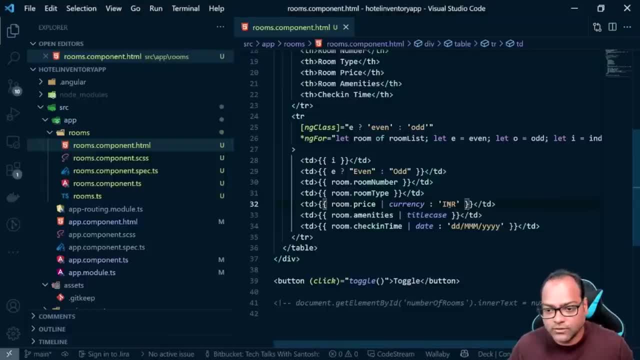 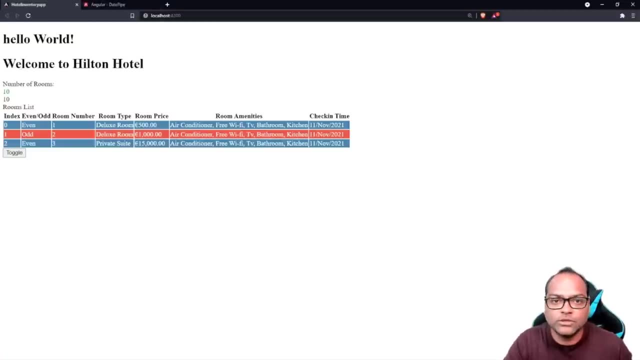 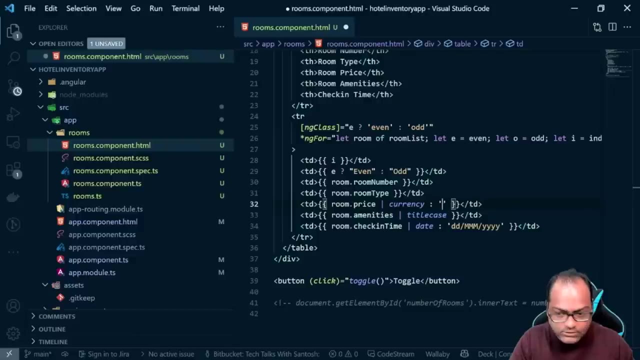 it will just display whatever you pass here. so here you have ionite, for example. if i want to display euro, i can say eur r, and it will display you the hero symbol. and uh, of course, a great britain pound, g, b, uh, gb, gb, and it will display the pound symbol. 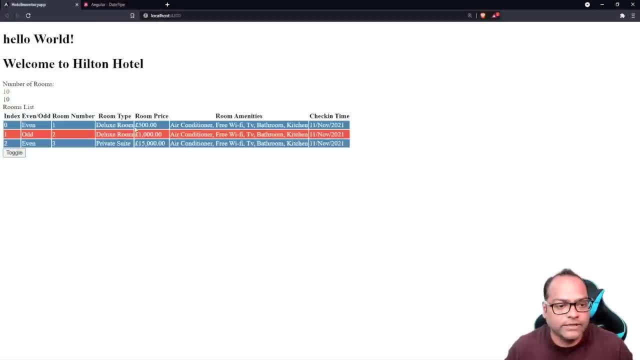 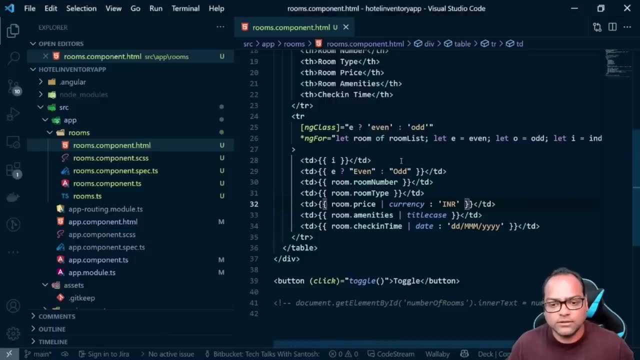 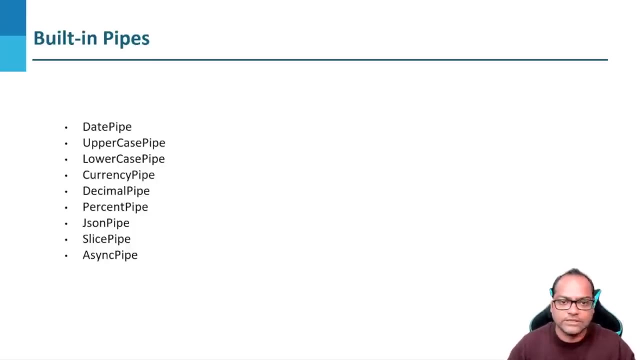 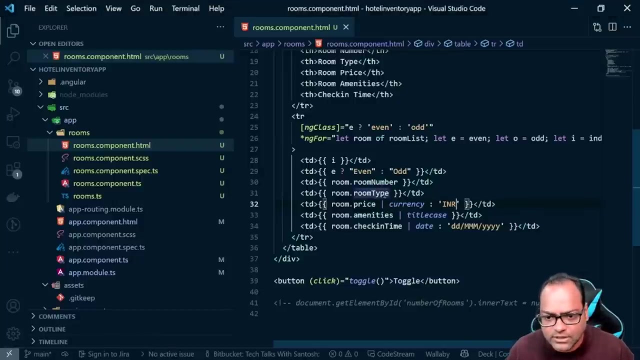 okay, saved, and you will get this pound symbol here, so by default it's you, but let's keep it as an inr. right now, indian rupees. so we are done. uh, we saw how trade pipe works, how we can use lowercase, uppercase, title case. then currency pipe. we have decimal and percentage pipe, so let's see percentage by first percentage. 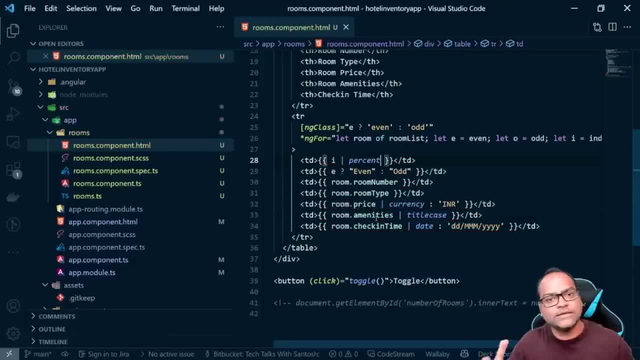 is uh, something which will display your value in person. so one is hundred percent. remember this. so, in case, uh, you want to actually uh convert some, some, some numbers in percentage, make sure that it is uh in decimal right. so let's go ahead and see, so you can see it is. 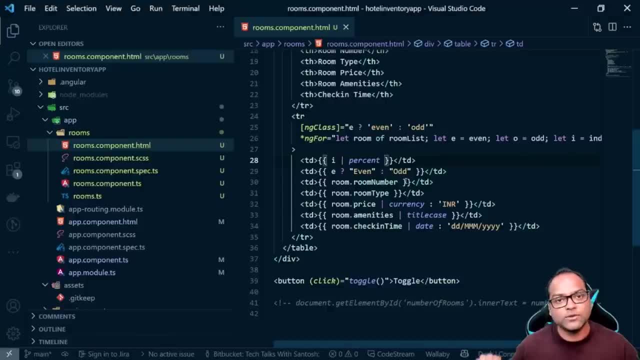 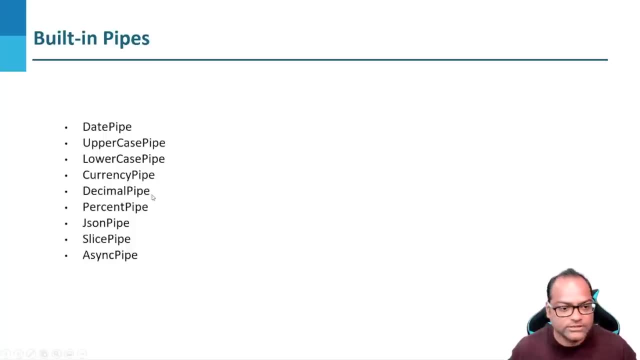 zero percent is a hundred percent and this is 200. so in case you have 0.5, it means 50, which is of course true, right? so, uh, this is percent pipe. we'll come back to decimal, and then we have json uh and uh slice, and and we have a sync pipe. so here we are going to say json pipe. 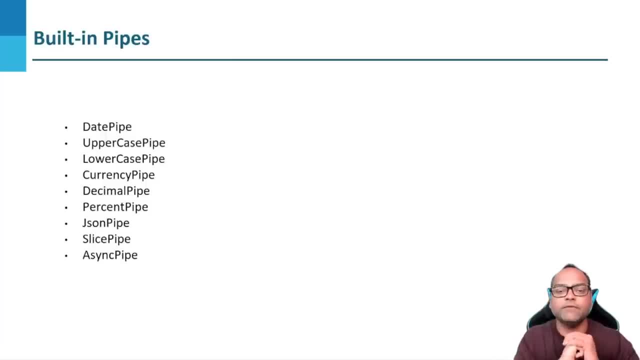 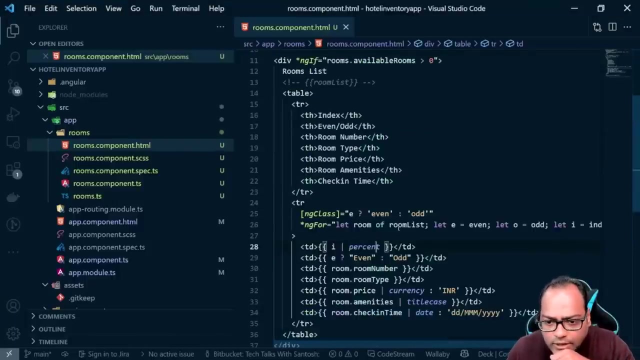 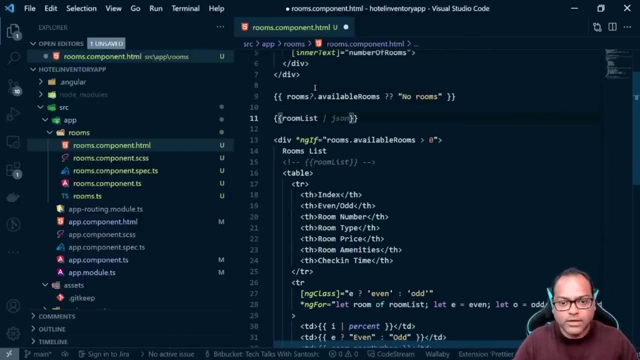 of course we will see slice paper as well. i think pipe we will not discuss right now. we will discuss it during uh, http and api calls. so we have to wait for that. let's see how to use this. so here uh room of room list. so json pipe is useful, uh, mostly for different purpose. for example, let's say this room list. 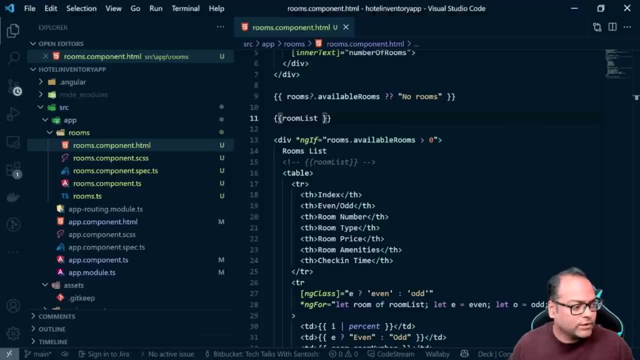 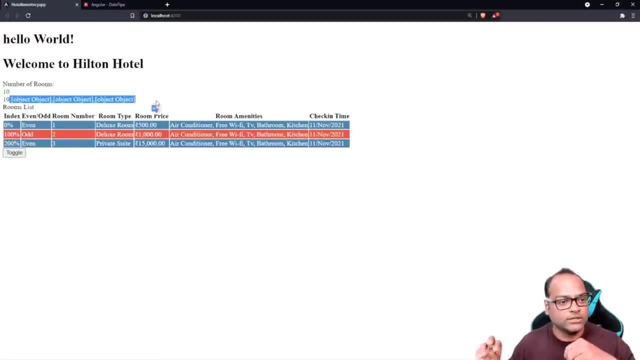 right, and it has a lot of objects, okay, a lot of other properties as well, and what you want to do is we want to just check what is the value available here. so if i just apply, or just apply these, uh, just apply this binding, you will see this is object, object. but what in case? i want to actually 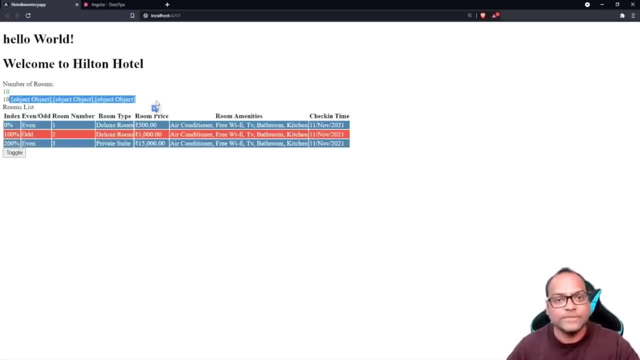 see the value, so i can just go ahead and write my code based on that. it happens because of course, we, in case you have large, largest object, you need to find, okay, which property exists and which property doesn't, so useful for deploying, don't keep json pipes on production. so let's see what. 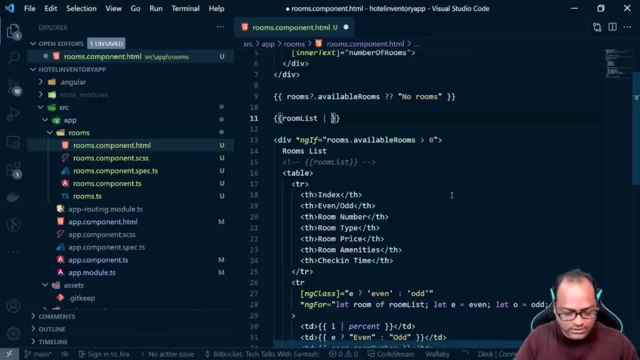 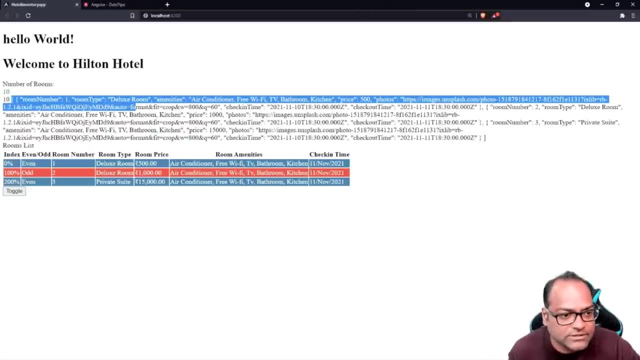 how json helps here. so i can just use five simple and can say: json, remember, it's all small. and now you can see: okay, okay, these are the values which are available. so it says: okay, there is a room number, there's a room type, these are the values. then you have photos object available as well. then you have check-in. 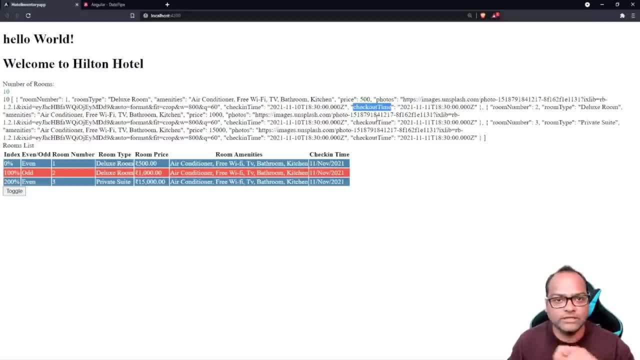 time check out. and these are all the properties which is available within this particular json property. it can be applied. it can be applied on object, it can be applied on an array, so you can apply it for everywhere. remember again, i am saying this is something which should be used for a. 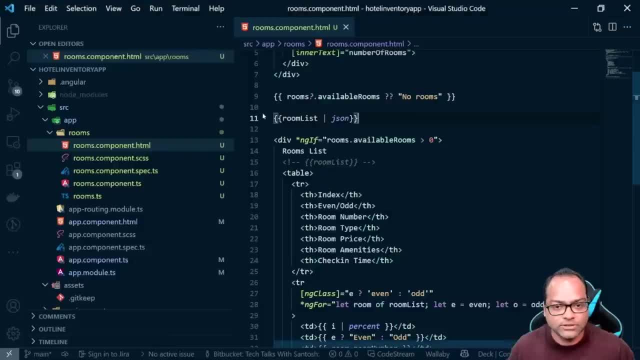 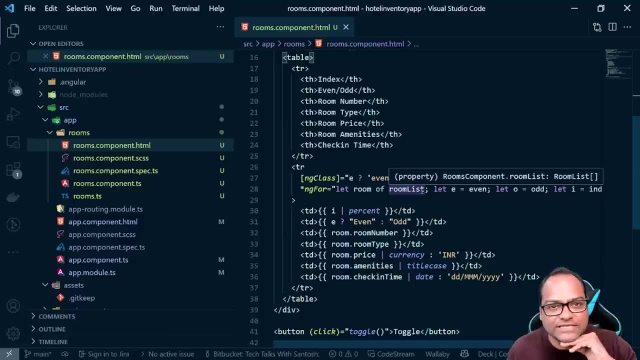 debugging purpose only, should not use on production. so this is json pipe. i'll just keep it here. i'll comment this. then we had slice pipe. so slice is similar to slice property, or you can say slice function, which exists in javascript. so here, uh, let's try to apply. 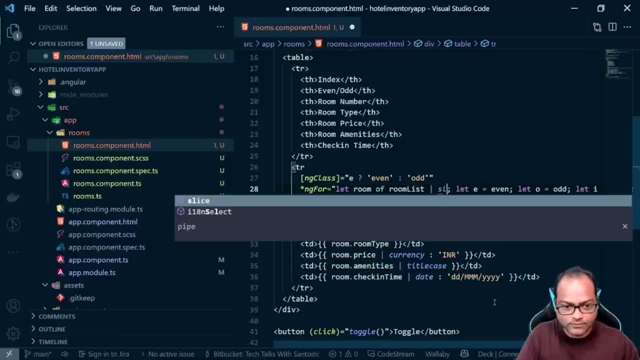 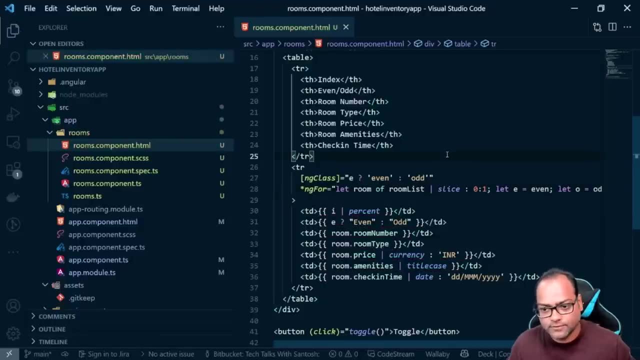 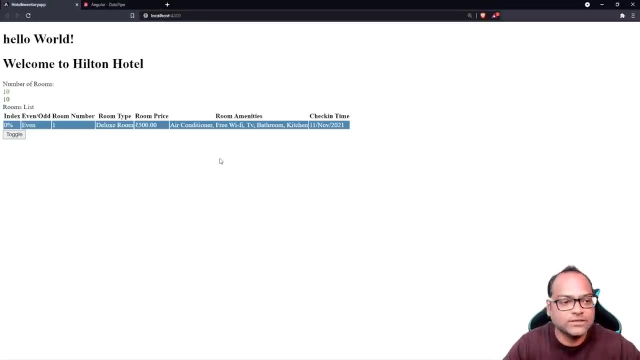 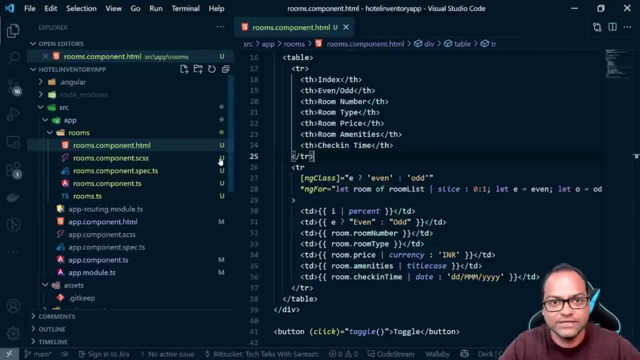 slice here and you can pass how many records you want to display. so i guess it's zero to one. so let's go ahead and see our view. you can see it says: okay, it displays first request because the pipe which we are using, the slice, or let's talk about slice function, which exists right. 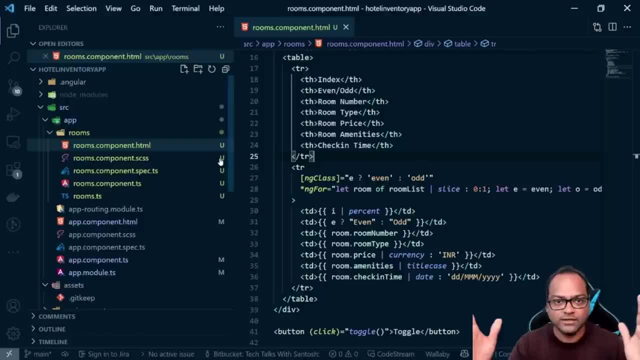 so slice function accepts two parameter, first index and the last index. it will display the value between that, those two. so here we are saying: start from the zero the index and display one value. you can also change, of course, uh, the first, and then you can say: okay, uh, go to. 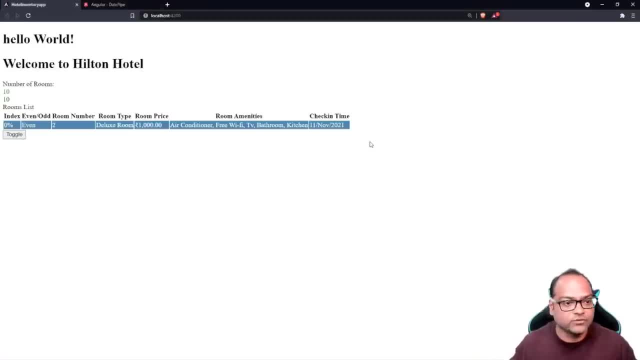 two right. so start from first and take the next two values. but doesn't exist. there are no other two values which exist, only there are zero, one, two. so it is only displaying me uh, the uh id. two right. so room number two, which is third record. so zero, uh, one, two. so between one. 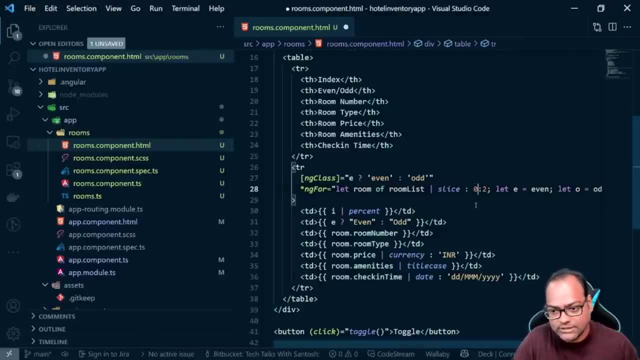 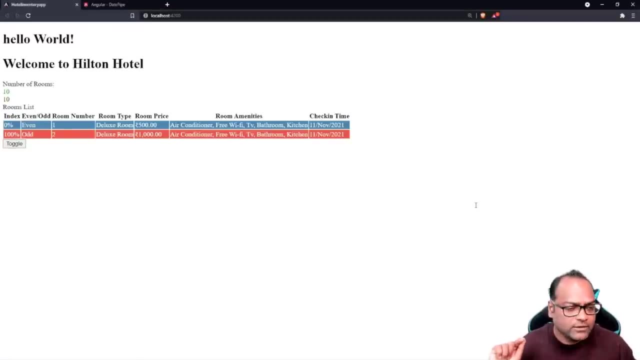 and two. there is only one record. if i say zero to two, let's see so it will always skip. if i am not wrong here, it will always skip zero and it will give you one. sorry, yeah, uh, sorry, i'm wrong. i'm wrong here. let's see the values. so you have uh room number one and two. right, so it will start. 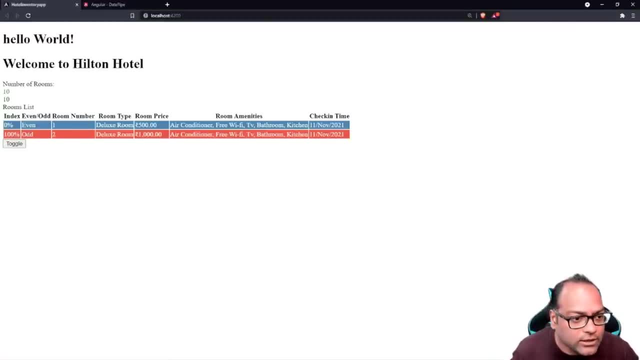 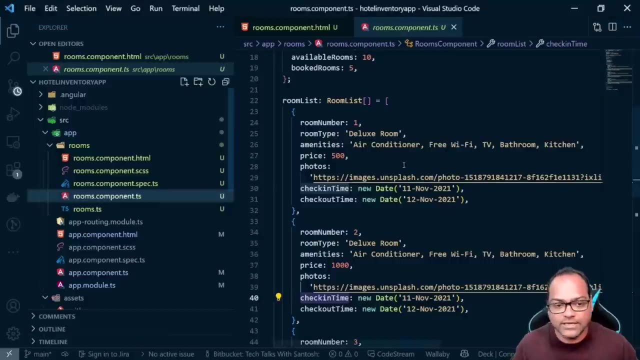 from zero and till two: zero one, two. so here, uh, so room number one and room number two. uh, it will skip the last one if i'm uh okay, so let's reiterate again, so when you pass slice and some numbers. so here what we are saying. 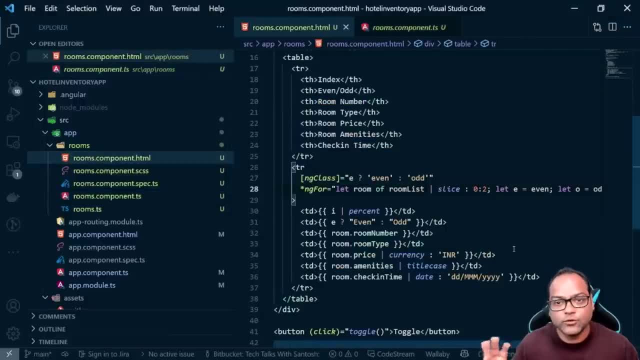 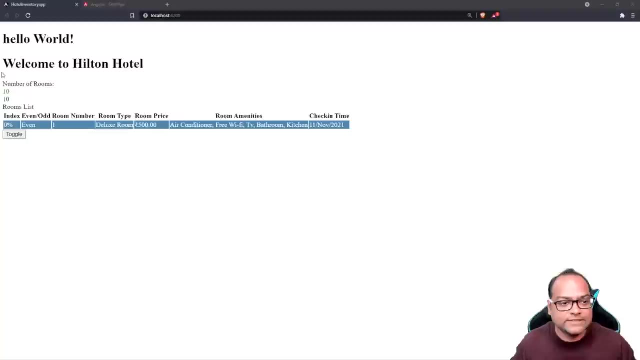 is starts from zero and go to go till two. so, uh, you have zero and one. it will not consider the last number. similarly, when we say zero and one, it will again skip the last number. so zero and one. and if i say zero to three, let's see what happens- it will, uh, display all the records, right, so zero. 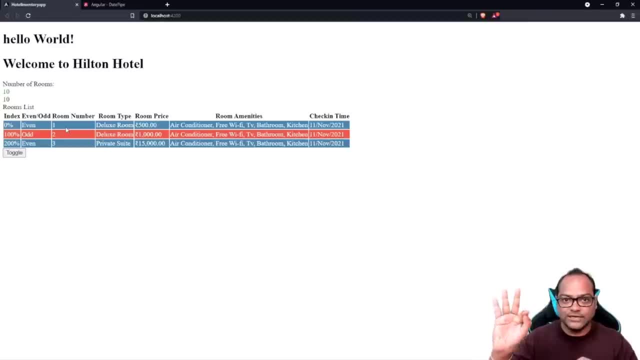 uh, because third index zero. uh, zero one, two, three. so third index is fourth value. so of course, there is nothing which exists there and it will always, uh, not consider the last, last value. so we get zero, one, two. similarly, when we passed two, what it did did is so zero, one and skip the last value, so zero and one. so this is how it. 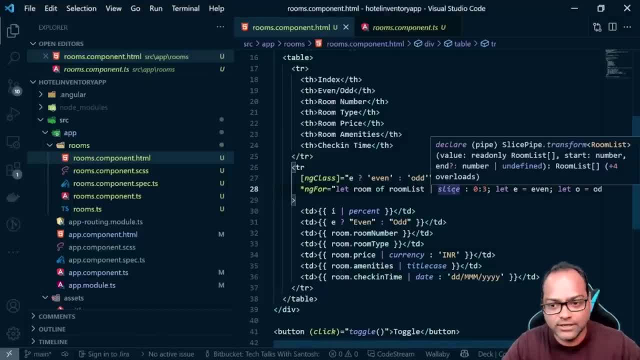 works. so, uh, generally you won't be using slice a lot of time because, in case you are working with large data set, it is not suggested that you should use slice pipe to filter out the records. so general i mean the use case to use slice pipe can be filtering without the records, but don't use it. 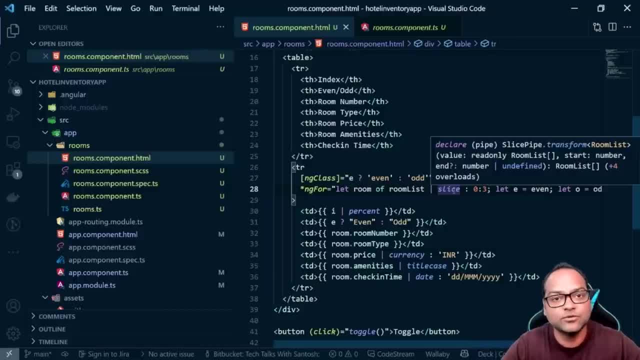 or you uh not filtering, sorry, uh, the general use case to use slices pipe? uh, sorry, general use case to you, uh, use slices pagination. so don't use the the slice pipe for pagination unless you have some like fixed records. so let's say you have some master table where, uh, your records are not going. 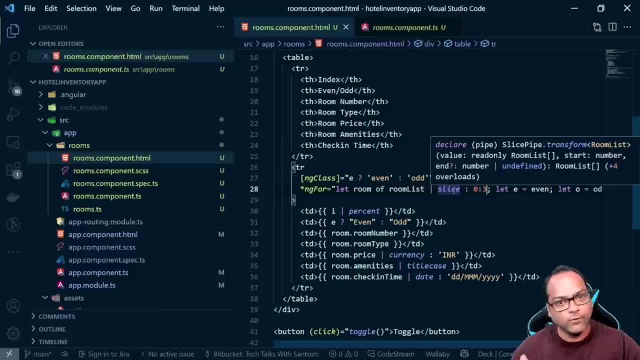 to go above five, fifty or, let's say, hundred. it will always be like that, which generally doesn't happen, right? i mean, most of the cases, you will get more. i mean, you don't know how many records we are supposed to get, so don't use slice for pagination in a real-time. 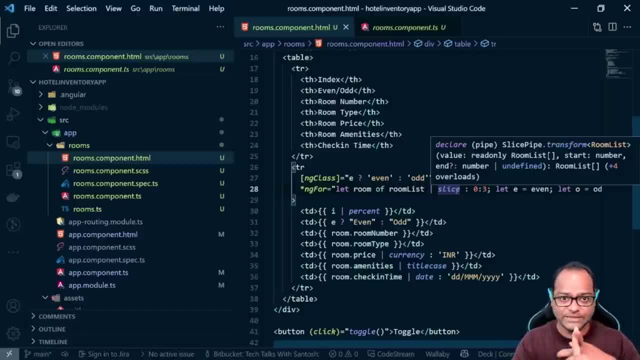 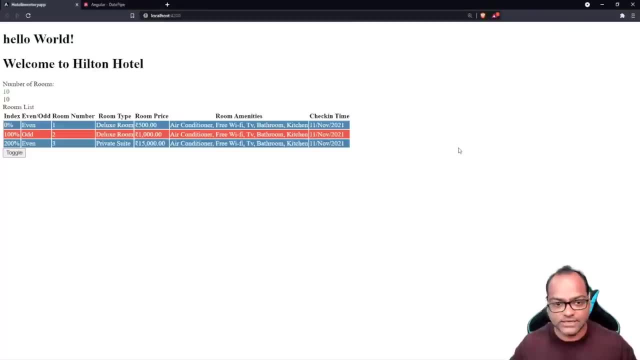 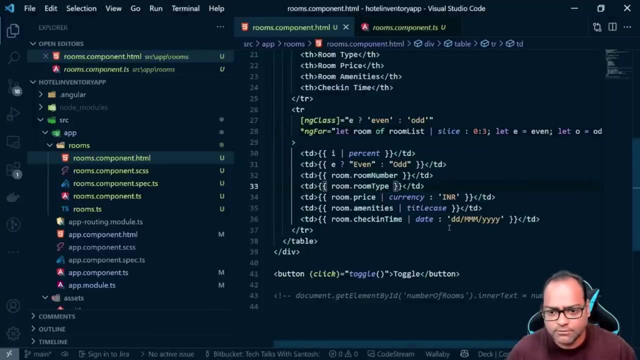 application always rely for server-side pagination or server-side filtering in case you are working with large data set. so this is a slice. and then we have number as well. so let's see if we get any more numbers here. so i don't have decimal numbers here. 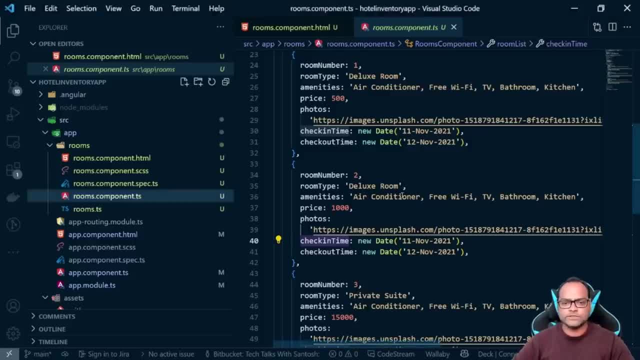 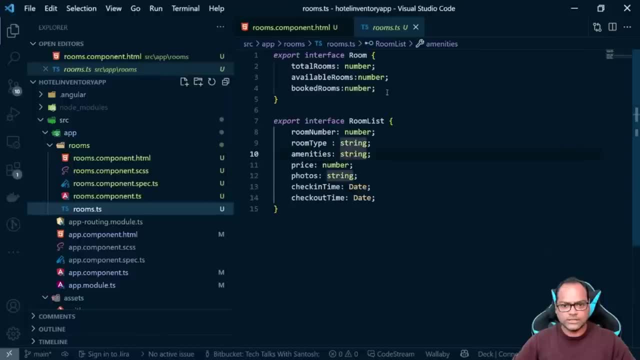 so for our decimal pipe example, right, so we are. what we will do is we will add one more property. so let's add a rating property, because that's something which can be decimal. so here i will say reading, and we will say: this is type of number. uh, you don't have like float here this uh. 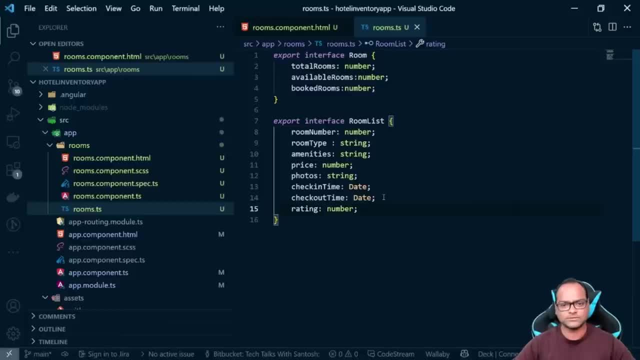 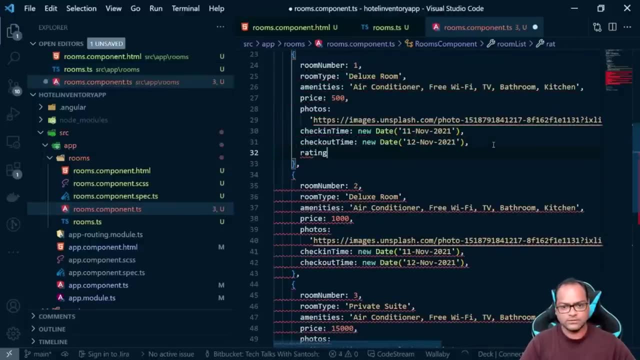 beacon does exist in typescript, but begin taste like for big numbers, so for writing i don't think so. we need uh begin, and now let's add this property. so i'll say this rating is uh 4.5 and here let's say it's 3.4. 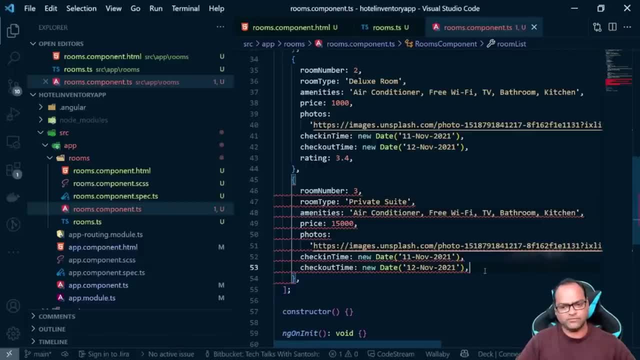 uh, this is out of 5, for example, and it says 2.6. so what we can achieve using decimal points. so let's say you don't want to actually round off these values or you don't want to round off these values to some specific numbers, so this is something which you can achieve using a decimal. 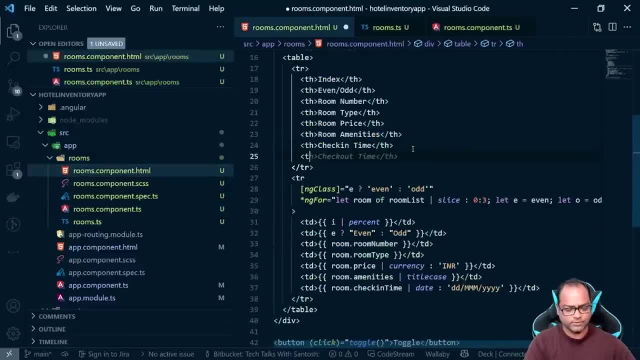 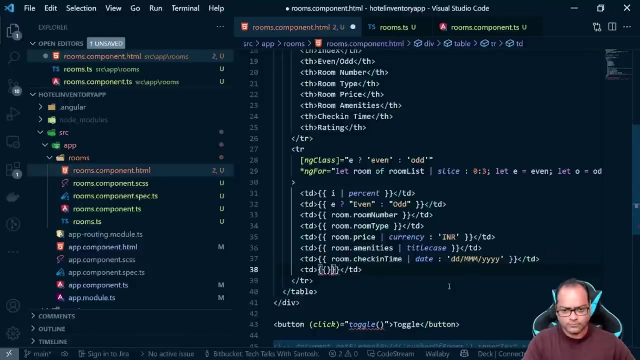 pipe. so here i'll just add a last property and i'll say: this is rating, so so room dot, so sorry. So let's apply decimal. sorry, not decimal. the name is decimal, but the bike name is number, So let's apply this and see how it looks like. 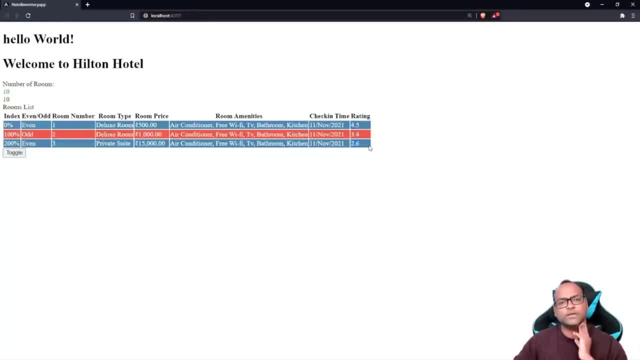 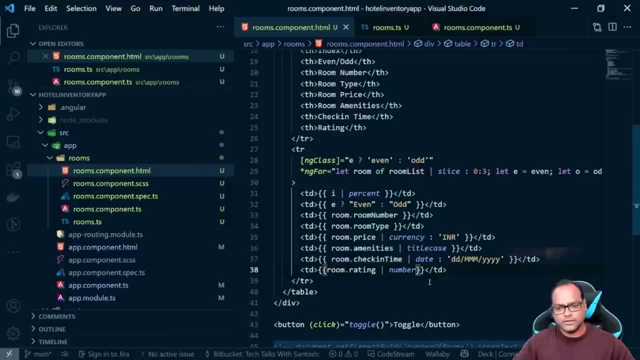 So you have this: 4.5, 3.5, 3.6,, for example. so this is the values, right, And now we want to actually display this in different format. So what we want is: there are three properties. there are three properties which you can pass. 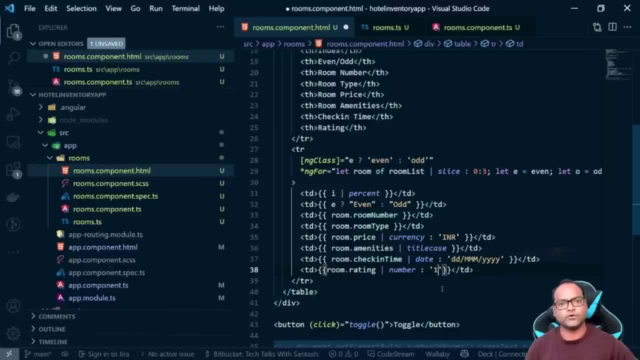 First is how many number we want to display before decimal. So I'm saying, okay, we want to display one number before decimal. Then how many decimals? sorry, how many numbers you want to display after decimals. For example, let's say zero and zero. 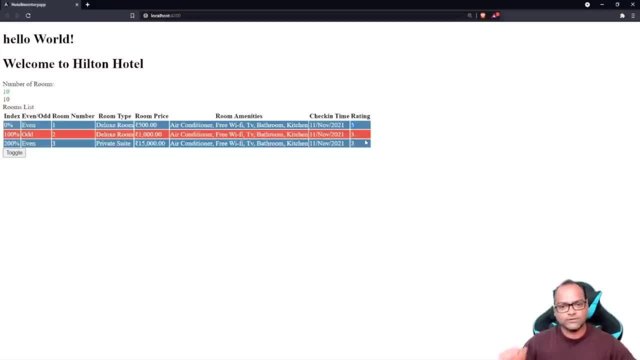 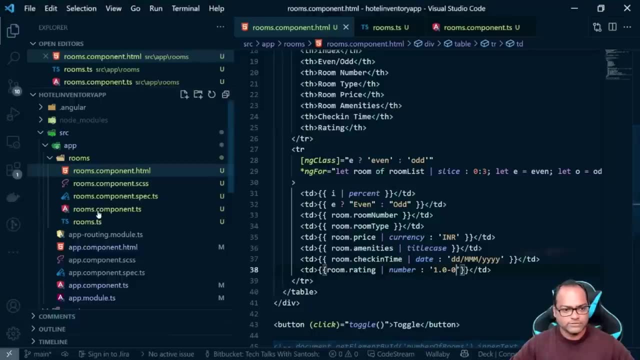 So it will. let's see what it does. So it says, okay, this 4.5 is closer to five, So it goes to five. Three point, I think. what were the other values? let's see. So we had 3.4 and 2.6.. 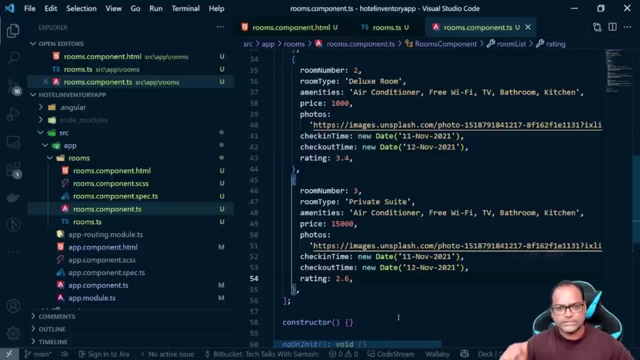 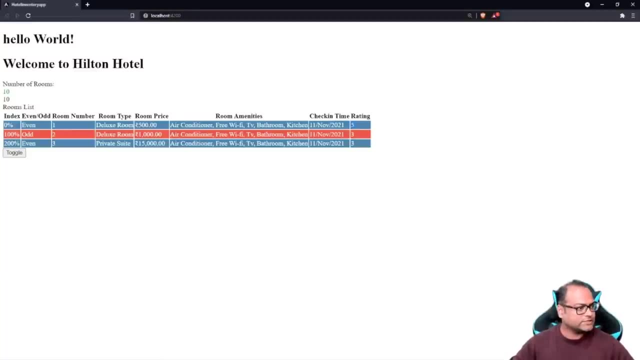 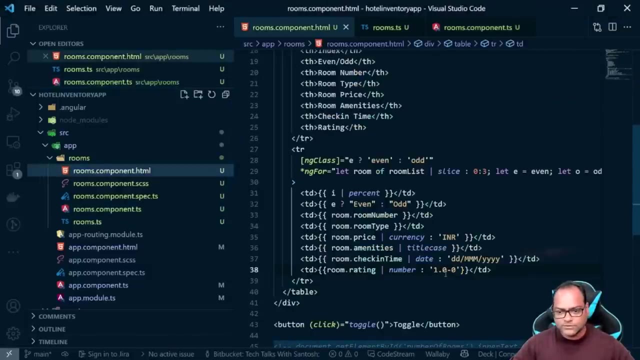 So 3.4 is closer to three, so it goes to three. 2.6 is closer to three, so it goes to three. So this is how this particular value works. Let's see how we can change the values. So this two values right. 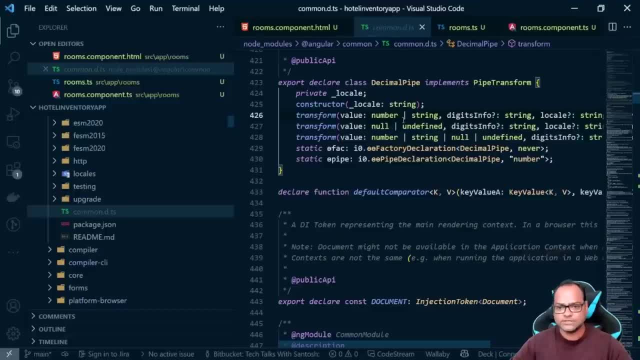 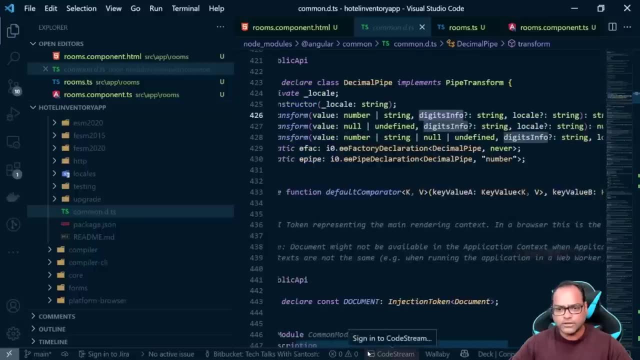 So this is minimum. you can actually see the definition here. so it says: this is the, this is the value and this is digits info And you can also pass local. but this is not we are looking at right now: decimal five. 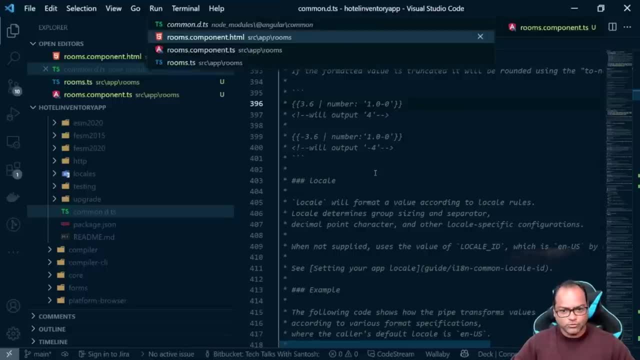 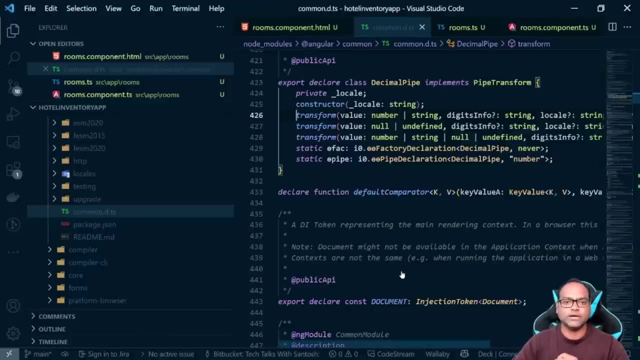 and here So you can see. let me show you the shortcut So you can actually go ahead and say control plus click. It will take you to this particular pipe in case it happens, right? So I generally don't use number pipe. 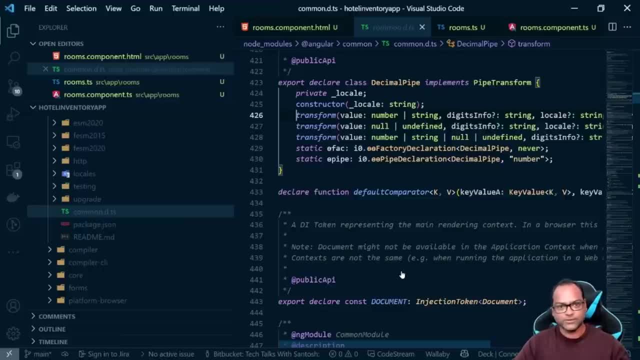 So if I forget about the definition, of course the docs is one place where I can see look for it, But you can also open this inside VS Code: Control plus, control plus, click here, or you can also do F12.. 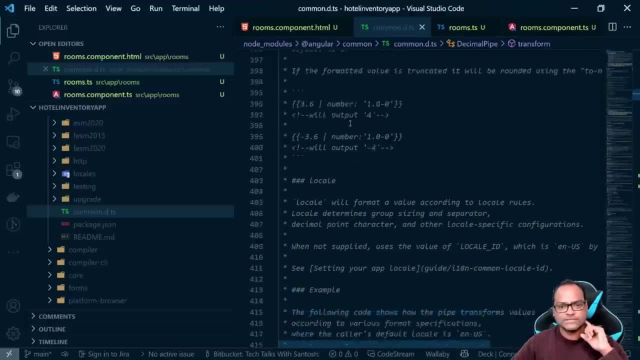 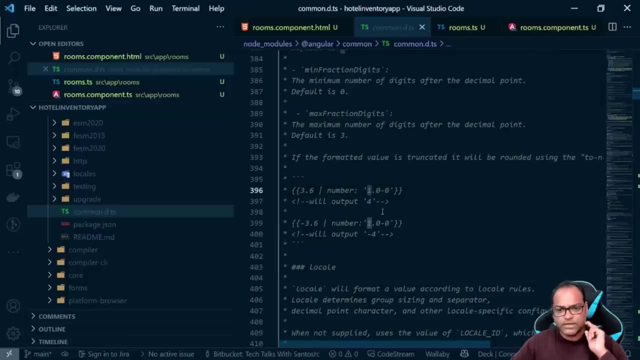 So press F12.. It will also take you to the definition file where you can see some example. For example, let's see here: So it says 3.6 number and we are saying first we want to display one number before the decimal. 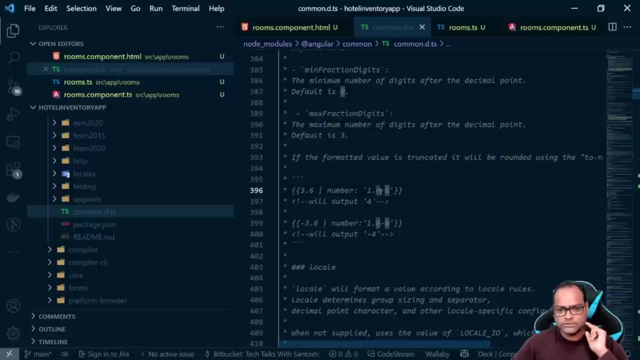 point, And after that we want to display a minimum zero, So you can see minimum number of digits after decimal point, So it says zero, and maximum number of digits after decimal point, So it says zero. So this is what we are saying. 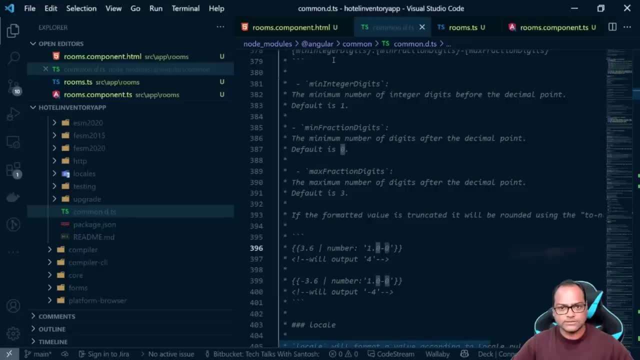 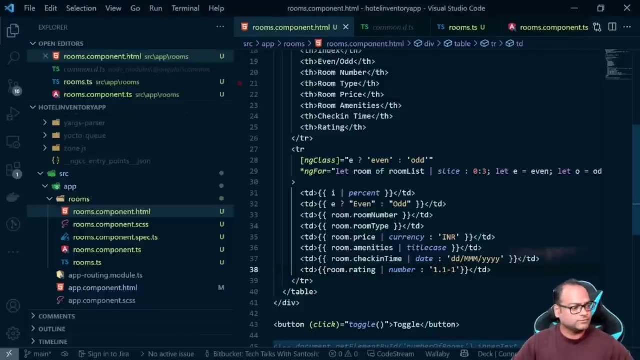 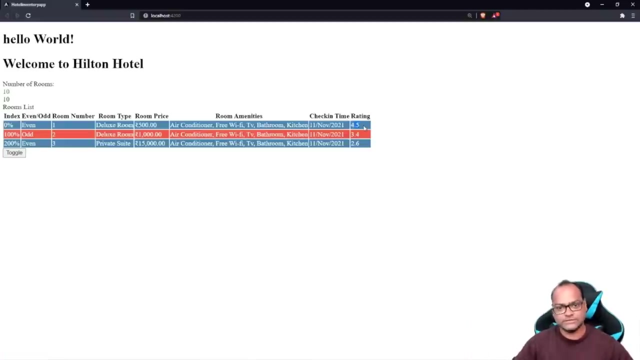 So let's say, if I do it like this, sorry, I want to display one and one, right? So we said, okay, we want to display at least one minimum digit and one maximum digit, which is four point, But in case we had a running number, right. 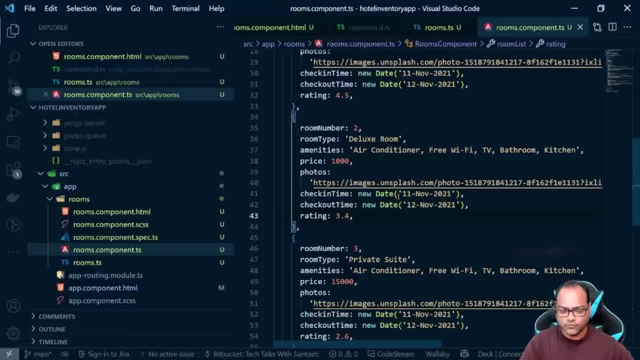 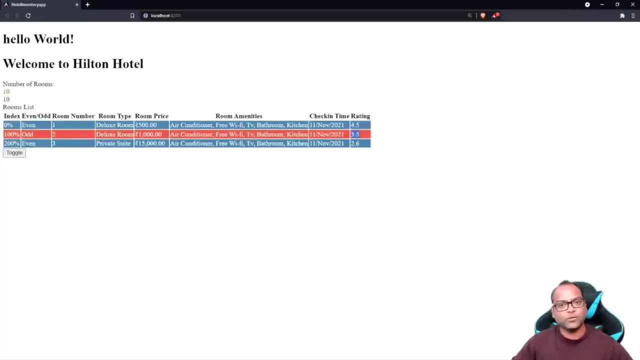 So let's say, if I change this to 3.4, where we have four, Okay, We have a few more numbers available. Now let's see what happens. So you have 3.5, because it actually said okay, 3.4, and we want to display only one. 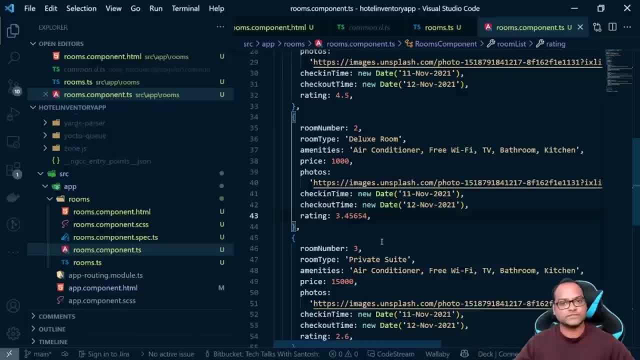 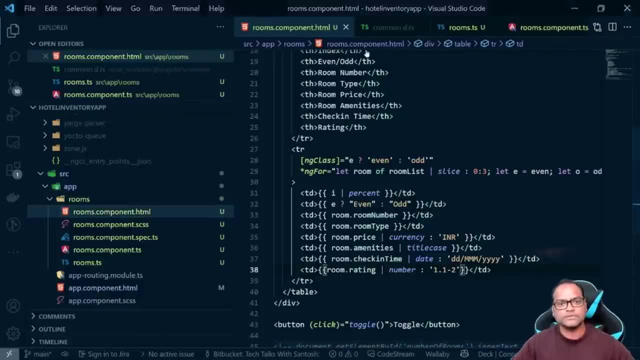 number. So it actually four is closer to five. So it says: okay, let's go to five and let's go to. I want to display two maximum numbers. Let's see what happens here. So you have 3.46.. 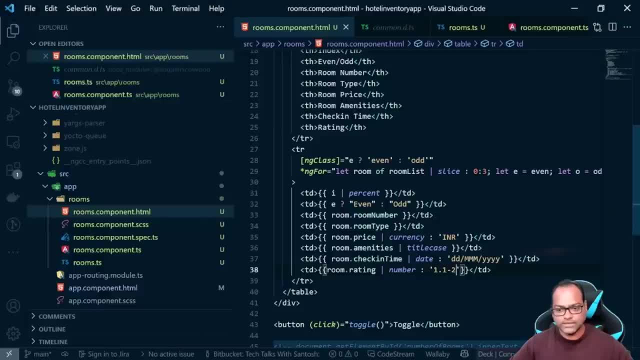 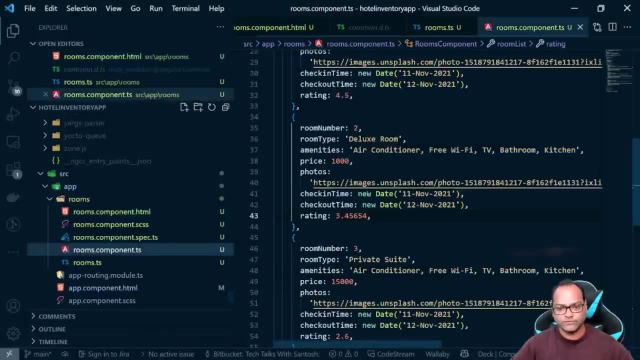 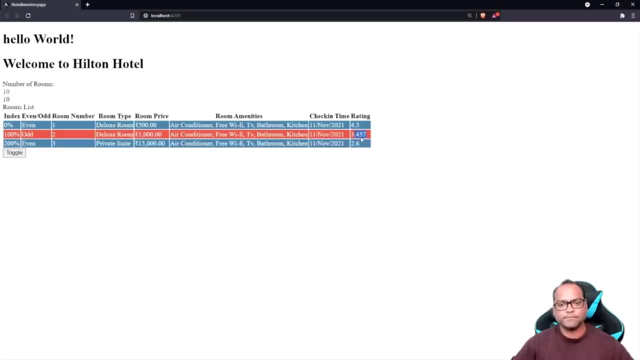 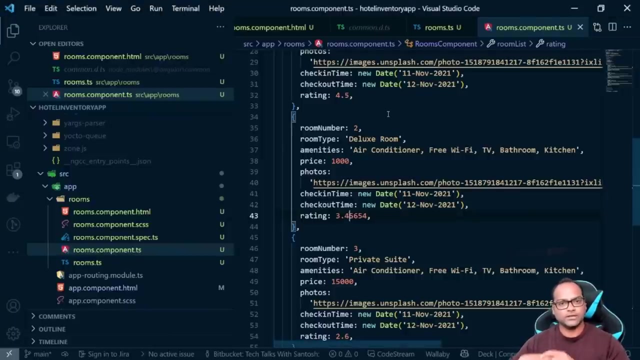 So this is two decimal numbers and we can, of course, increase to whatever maximum numbers you want to. So now you have 3.4.457.. So this is how you can actually use this number Right, And you can also pass local, which is, like you remember, the numbers are actually different. 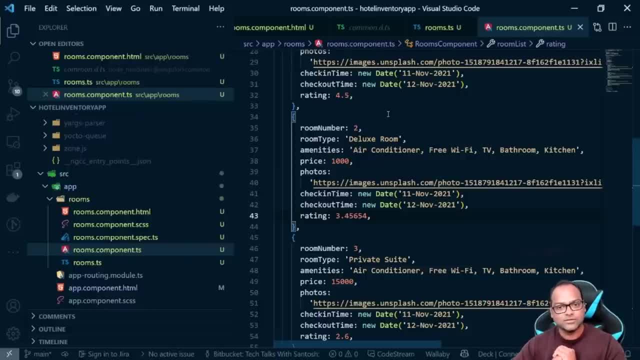 in different countries. So, for example, here in India we use decimal points, But if you go to Europe sometimes they use complex numbers. So, for example, here in India we use decimal points, But if you go to Europe sometimes they use complex numbers. 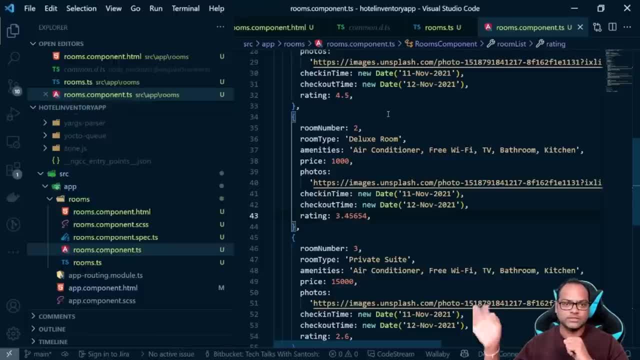 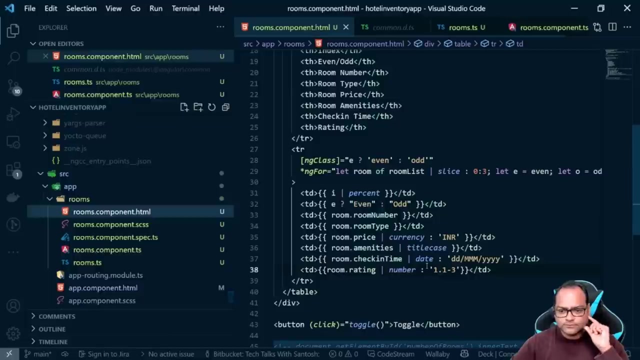 But if you go to France they use comma, Or probably some other countries might be using some other different separation value, So different separator, which you call, You can also do that using this. Let me see if there's any samples. So let's try to display this number in France. 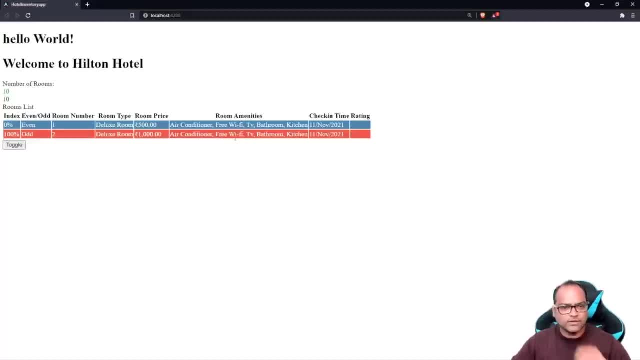 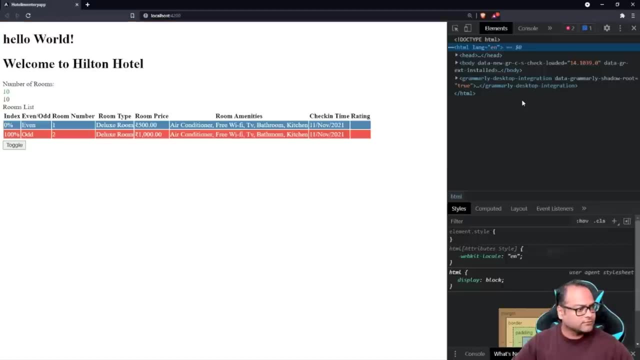 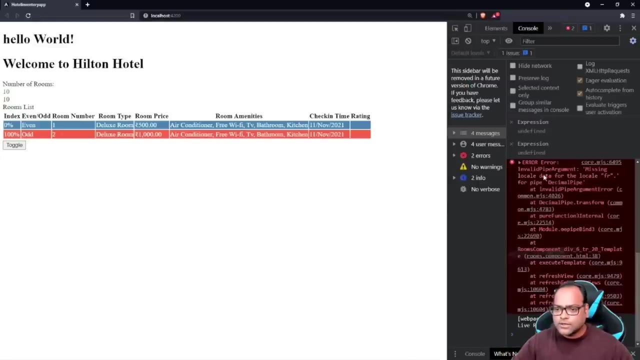 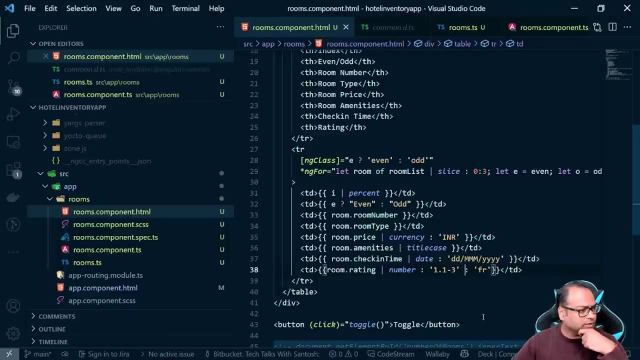 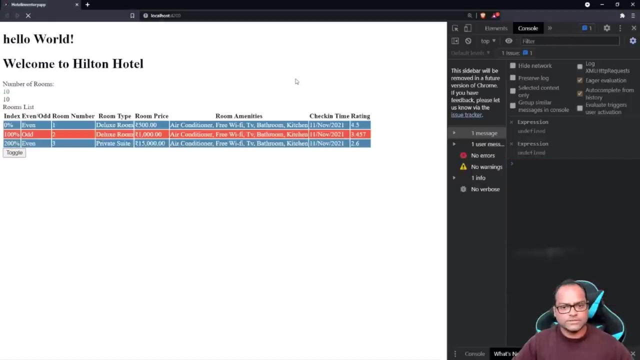 Okay, dfr is local for france. let's see. okay, there is some error. okay, this is not something which is valid local. invalid pipe argument: missing local data for? uh? okay, missing the local data. so we have to add local first and then it's okay. let's see, en us is available. yes, this is available and this is the default one. 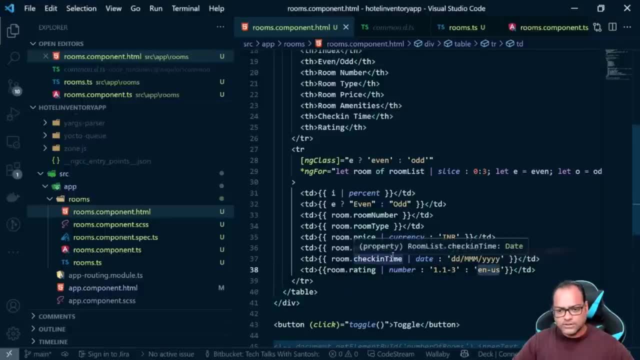 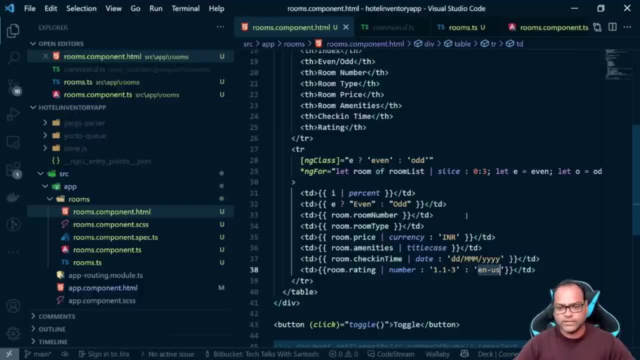 that's, that is something which is not added. that's, that is something which is not added. probably we'll see an example. uh, probably we'll see an example. uh, probably we'll see an example. uh, i'll later on. but yeah, i mean you can, i'll later on, but yeah, i mean you can. 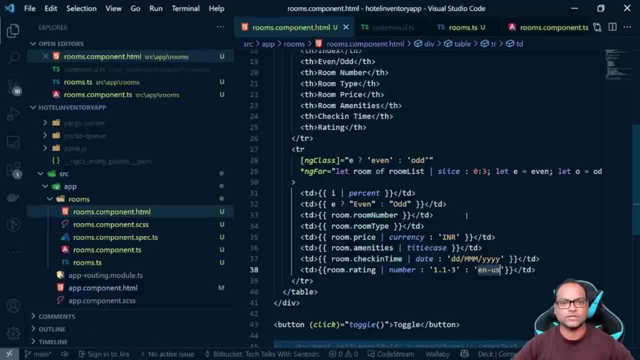 i'll later on. but yeah, i mean you can pass the locals here and then it will pass the locals here, and then it will pass the locals here and then it will display the number based on that display, the number based on that display, the number based on that particular local. so 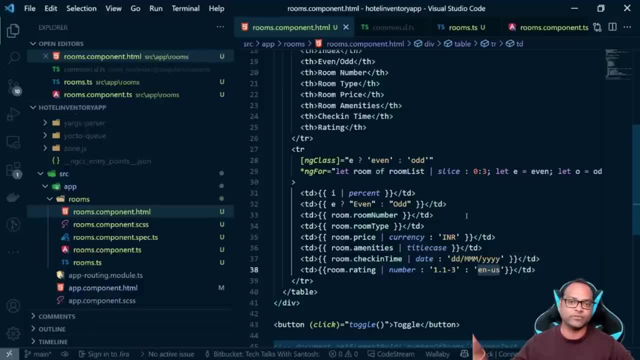 particular local, so particular local, so, for example, this number may be different. for example, this number may be different. for example, this number may be different, or in a different format in france, which, or in a different format in france, which, or in a different format in france, which is possible and it is possible. let's 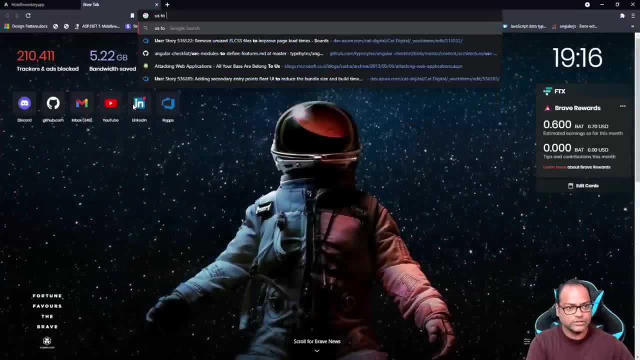 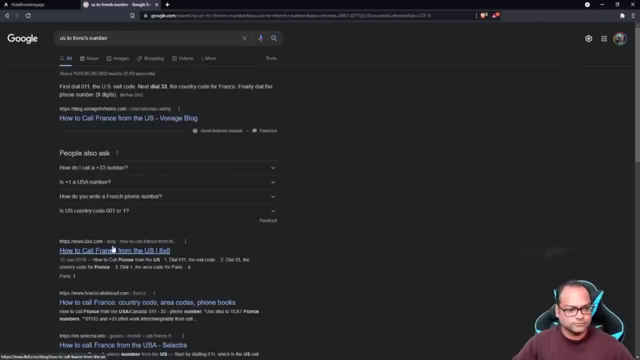 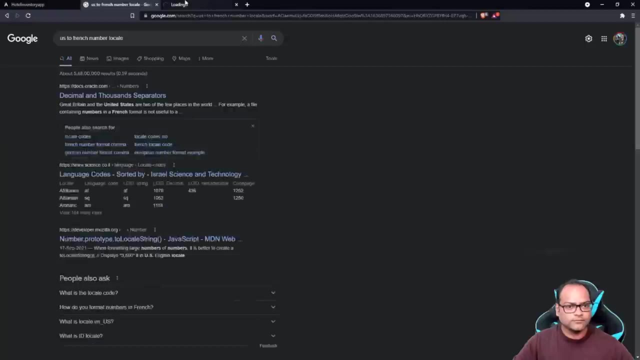 is possible and it is possible. let's is possible and it is possible. let's call it, call it. call it plus plus plus two, so you can see thousand and decimal. so you can see thousand and decimal. so you can see thousand and decimal. separators, right so. separators, right so. 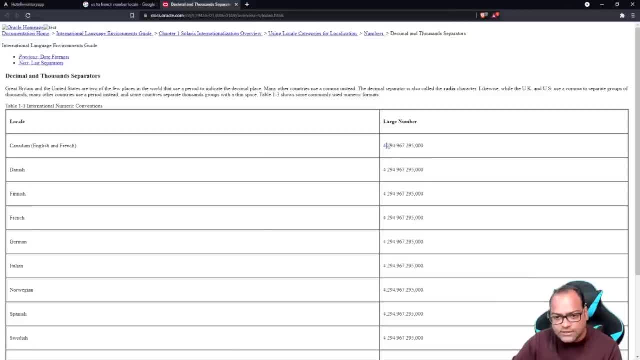 separators. right. so uh in canada, you uh, we use space. uh in canada, you uh, we use space. uh in canada, you uh, we use space in danish, where you are in danish, where you are in danish, where you are. uh, uh, we are using space. so in different currencies. 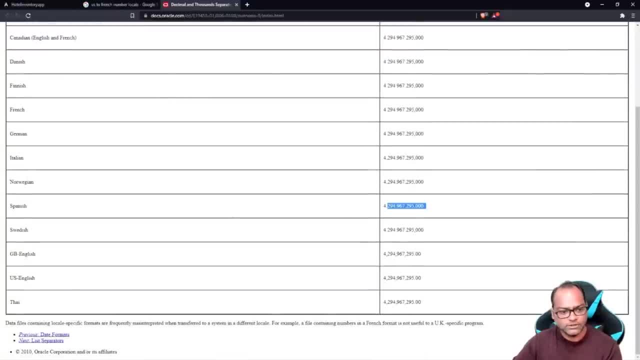 we are using space, so in different currencies we are using space, so in different currencies, there are different separators which are used. there are different separators which are used. there are different separators which are used. so this is what i was referring to. so, this is what i was referring to. 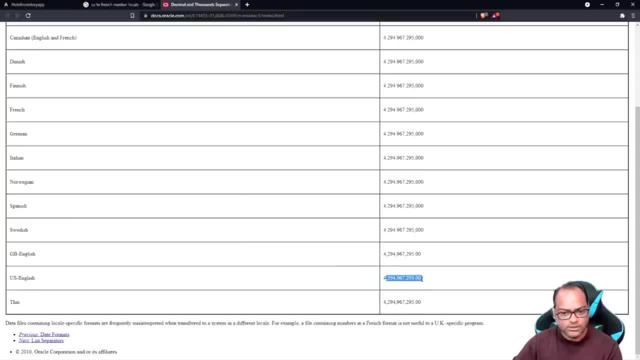 so this is what i was referring to. so thai, you have comma, then dot, so thai. you have comma, then dot, so thai you have comma, then dot. here also you have comma spanish there. here also you have comma spanish. there, here also you have comma spanish. there is no comma, there is just spaces. 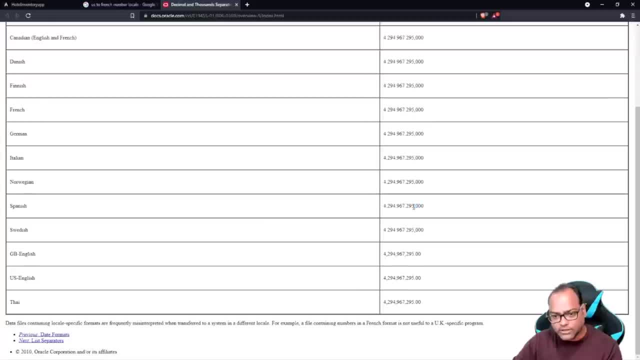 is no comma, there is just spaces- is no comma, there is just spaces. i'm sorry, space, you have dots and i'm sorry, space, you have dots and i'm sorry space you have dots. and then dot- here you have comma, so these. then dot, here you have comma, so these. 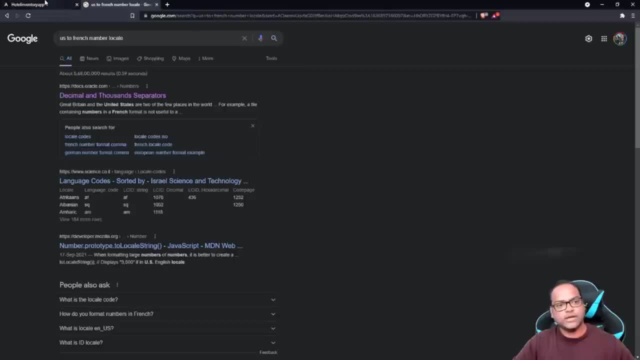 then dot. here you have comma. so these are different. uh numbers format in are different uh numbers format in are different uh numbers format in different locals, different locals, different locals. and angular supports different locals as and angular supports different locals as and angular supports different locals as well. i mean, that's another. 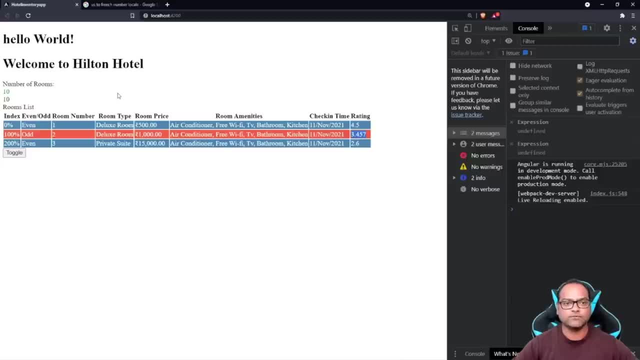 well, i mean that's another. well, i mean that's another topic uh, which is not part of this course. topic uh, which is not part of this course. topic uh, which is not part of this course, but in case you want to refer, but in case you want to refer, 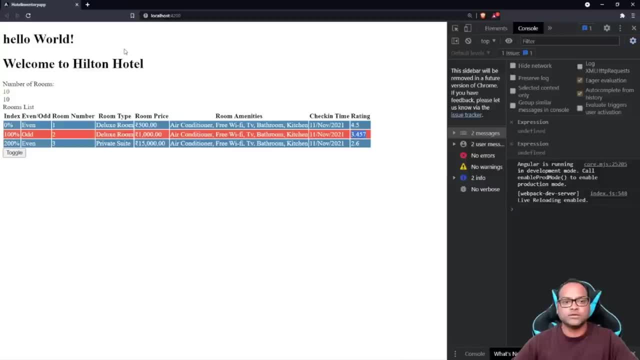 but in case you want to refer uh angular does support uh converting uh angular does support uh converting uh. angular does support uh converting your, your, your, uh like, uh like, uh like text to a different format, which is text to a different format, which is text to a different format, which is known as internet internationalization. 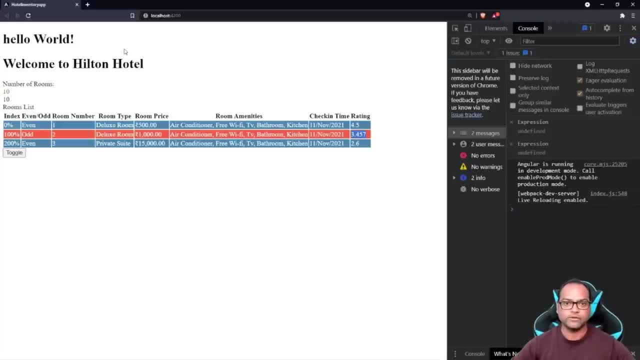 known as internet internationalization, known as internet internationalization and localization. it is a feature which, and localization. it is a feature which, and localization. it is a feature which is up which is supported by angular, is up which is supported by angular, is up which is supported by angular. so that's it from the pipes as we 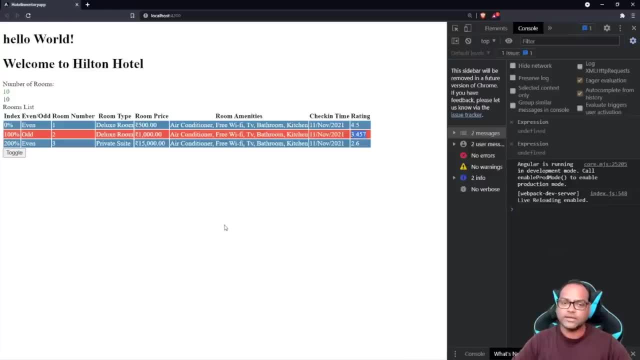 so that's it from the pipes as we. so that's it from the pipes as we mentioned. the sync pipe will be used. mentioned: the sync pipe will be used. mentioned: the sync pipe will be used while talking about http in the next. while talking about http in the next. 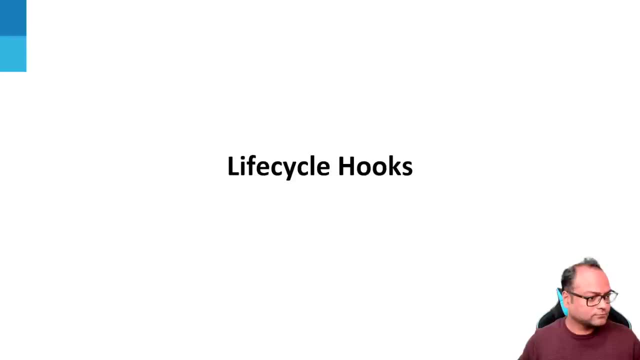 while talking about http in the next section, hi in this video we are going to talk hi in this video, we are going to talk hi in this video, we are going to talk about lifecycle looks, about lifecycle looks, about lifecycle looks. but before we do that, let's do one more. 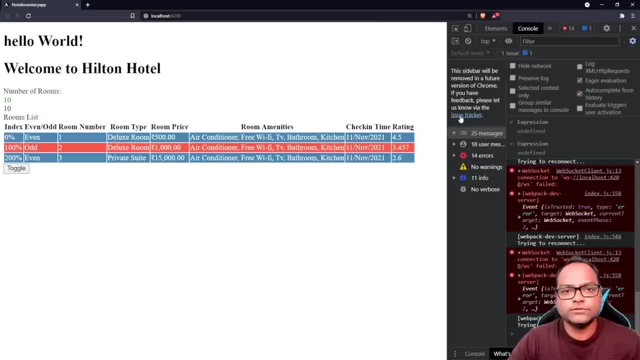 but before we do that, let's do one more. but before we do that, let's do one more thing right now. if you see this particular view right now, if you see this particular view right now, if you see this particular view, it's missing something. it is missing. 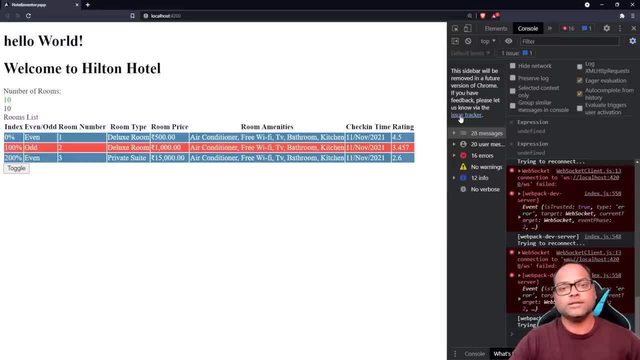 it's missing something. it is missing. it's missing something. it is missing the styling, if you think about it right. the styling if you think about it right. the styling if you think about it right. so there are multiple options which you, so there are multiple options which you. 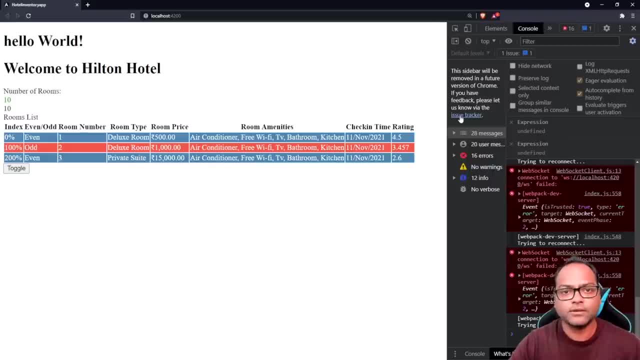 so there are multiple options which you can choose from. can choose from. can choose from: you can either go with bootstrap, you can either go with bootstrap. you can either go with bootstrap, you can go with angular material, or you you can go with angular material, or you you can go with angular material, or you can also use. 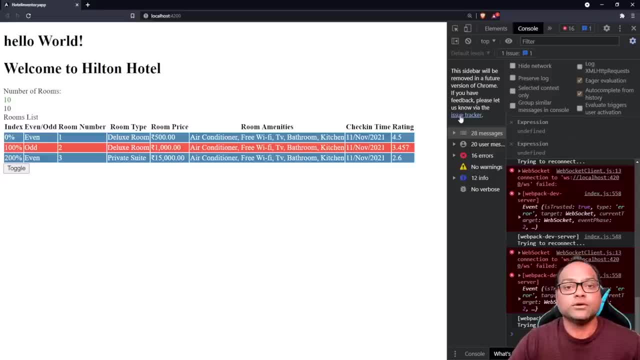 can also use, can also use something. uh, or you can also use, or you can also use, or you can also use tellwind css, which is also supported by tellwind css, which is also supported by tellwind css, which is also supported by angular, angular, angular. so what we will do is let's add bootstrap. 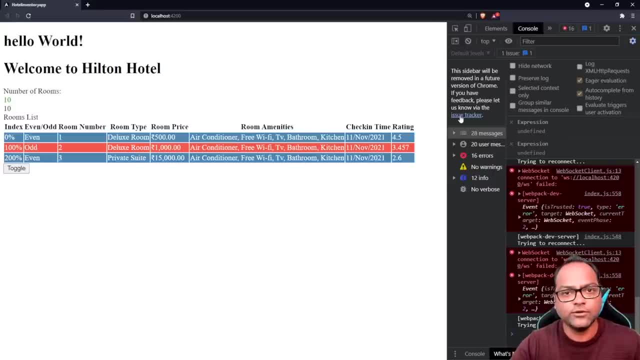 so what we will do is: let's add bootstrap. so what we will do is: let's add bootstrap right now and right now and right now, and then we will add angular material later, then we will add angular material later, then we will add angular material later on. 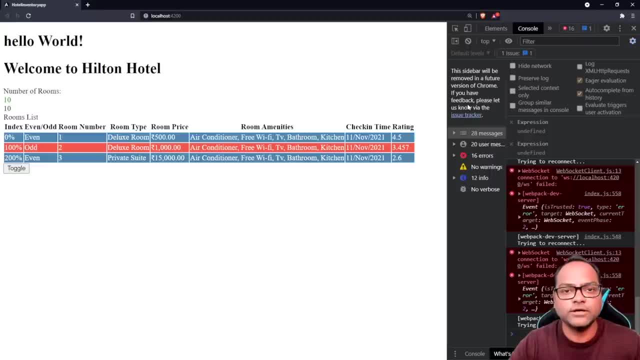 on on and probably at the end we will see how, and probably at the end we will see how, and probably at the end we will see how you can configure. you can configure, you can configure tellwind css, probably later in the video. tellwind css- probably later in the video. 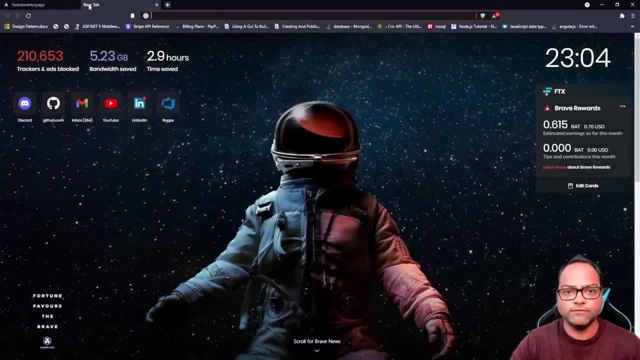 tellwind css, probably later in the video. so to add bootstrap. there are multiple. so to add bootstrap. there are multiple. so to add bootstrap. there are multiple options which you have. there are multiple options which you have. there are multiple options which you have. there are multiple libraries which actually supports. 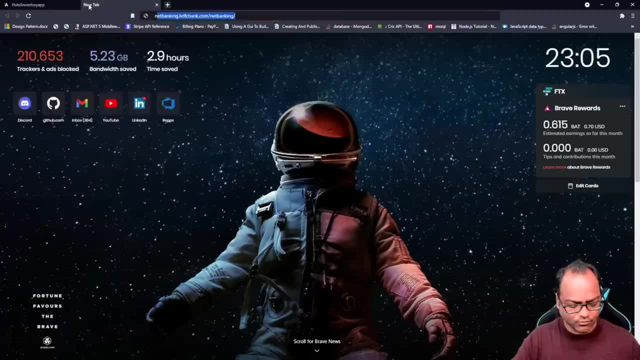 libraries, which actually supports libraries, which actually supports bootstrap, bootstrap, bootstrap. so we have ngx bootstrap and ng. so we have ngx bootstrap and ng. so we have ngx bootstrap and ng bootstrap. both are same bootstrap, both are same bootstrap. both are same. even contains a lot of similar. even contains a lot of similar. 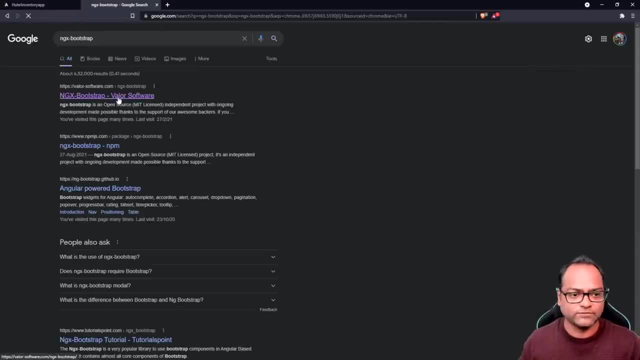 even contains a lot of similar components. i mean you can choose anyone. components. i mean you can choose anyone. components, i mean you can choose anyone. they both support bootstrap 4 as of now. they both support bootstrap 4 as of now. they both support bootstrap 4. as of now, they don't have support for bootstrap 5. 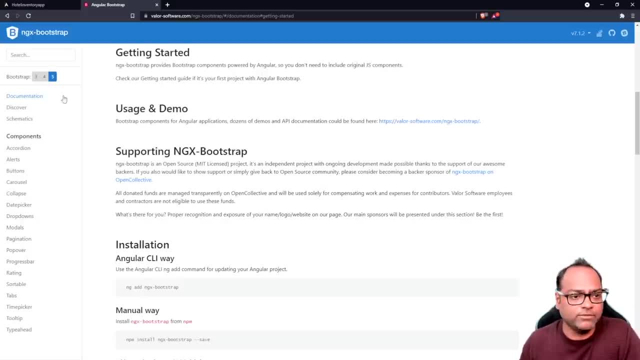 they don't have support for bootstrap 5. they don't have support for bootstrap 5, so let's see. okay, so ngx bootstrap, so let's see. okay. so ngx bootstrap. so let's see. okay. so ngx bootstrap. actually came with, suppose he came up. actually came with, suppose he came up. 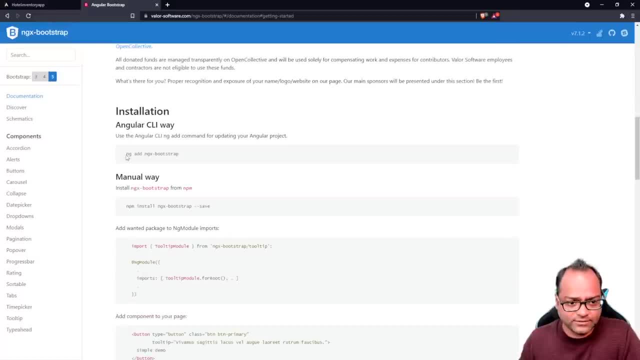 actually came with, suppose he came up with the support for bootstrap fiber also, with the support for bootstrap fiber, also with the support for bootstrap fiber also. so let's add, so, let's add, so, let's add. you can add this command. you can see um. you can add this command. you can see um. 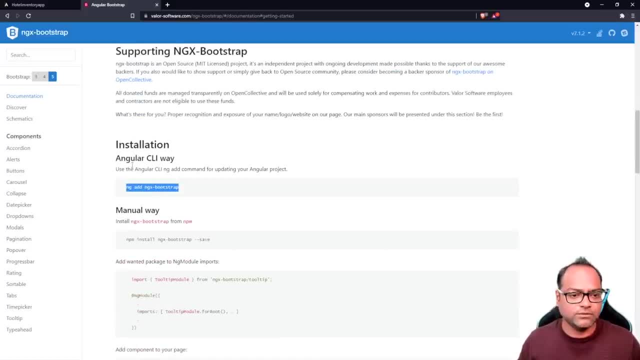 you can add this command. you can see um how you can install. so there are how you can install. so there are how you can install. so there are instructions given on this page. uh you, instructions given on this page. uh you, instructions given on this page. uh you, we can. we will use the angular cli way. 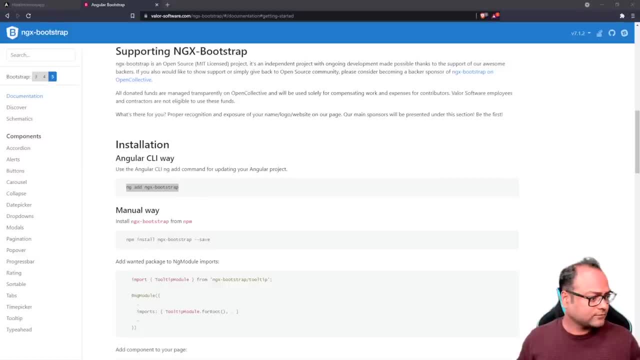 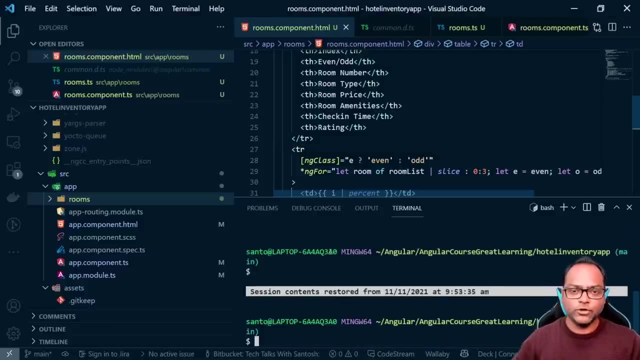 we can, we will use the angular cli way. we can, we will use the angular cli way. so let's go ahead and do that, and before you do that and before you do this, make sure you, and before you do this, make sure you, and before you do this, make sure you stop the server which is running. so 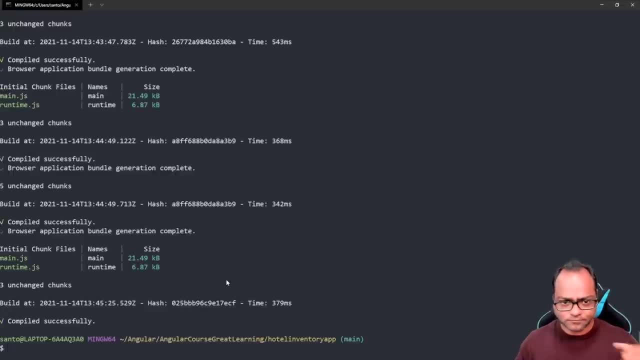 stop the server which is running. so stop the server which is running. so i have stopped the server because it is. i have stopped the server because it is. i have stopped the server because it is going to impact, going to impact, going to impact the angularjson and we need to restart. 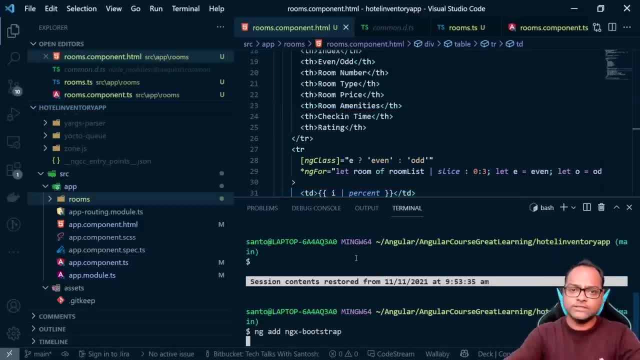 the angularjson and we need to restart the angularjson and we need to restart the server. so the server, so the server. so i already stopped it. in case you are, i already stopped it. in case you are, i already stopped it. in case you are running, just stop and. 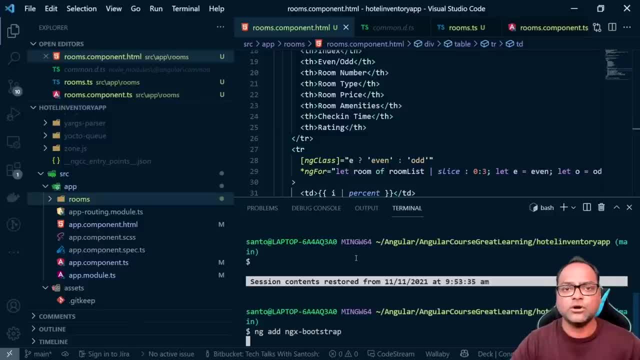 running. just stop and running. just stop and run this command: ng add njx bootstrap. run this command: ng add njx bootstrap. run this command: ng add njx bootstrap, which will install bootstrap 5, which will install bootstrap 5, which will install bootstrap 5 and it will give access to some. 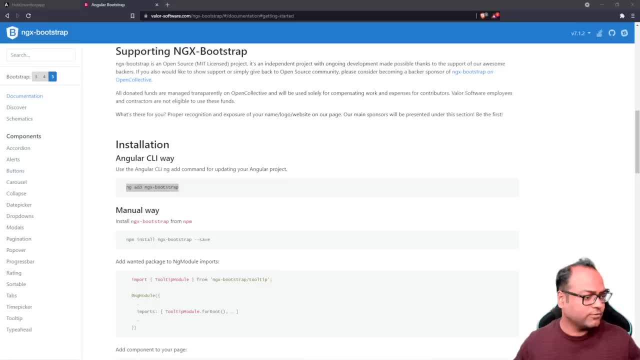 and it will give access to some. and it will give access to some components which comes with it. so if components which comes with it, so if components which comes with it, so if let's go back to the page so you can, let's go back to the page so you can. 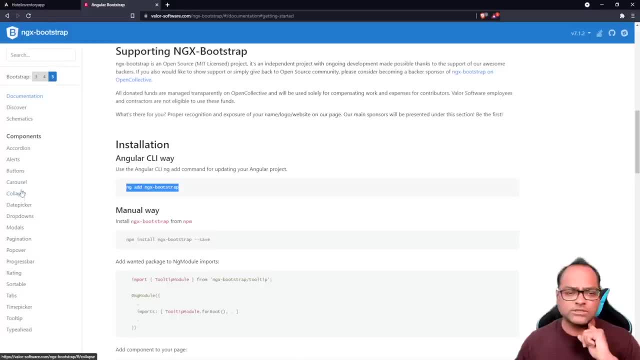 let's go back to the page so you can see it has accordion alerts button. see it has accordion alerts button. see it has accordion alerts button- carousel collapse, carousel collapse, carousel collapse. so these are all components which you so, these are all components which you so, these are all components which you, you can use inside your. 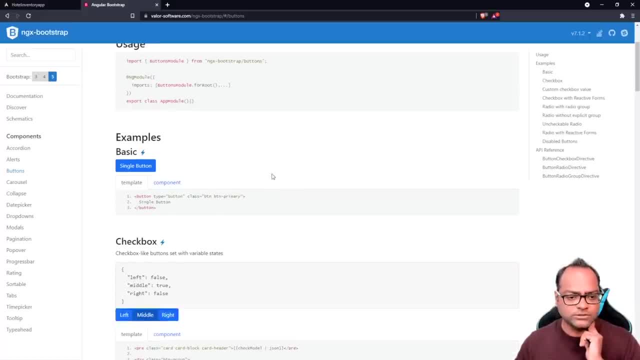 you can use inside your. you can use inside your angular page or angular application, angular page or angular application, angular page or angular application. so we'll. we'll come back to this later. so we'll. we'll come back to this later. so we'll. we'll come back to this later on. right now, we just want to install. 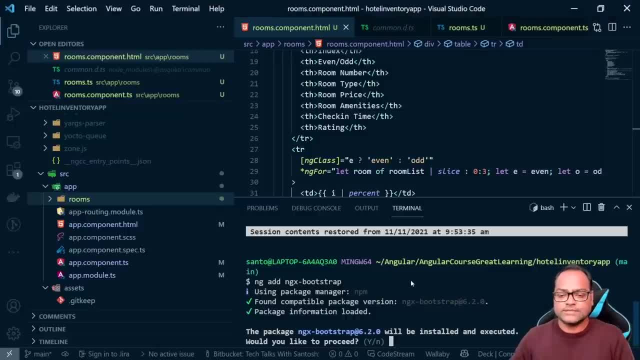 on right now. we just want to install on right now. we just want to install njx bootstrap, so njx bootstrap, so njx bootstrap. so let's see, it says: uh, the package ng, let's see. it says, uh, the package ng, let's see. it says, uh, the package ng bootstrap 6.2.0 will be installed. and. 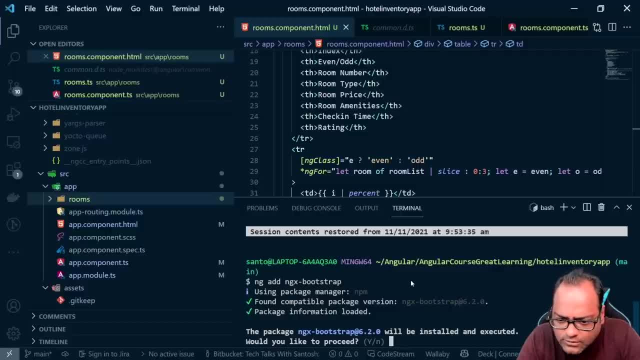 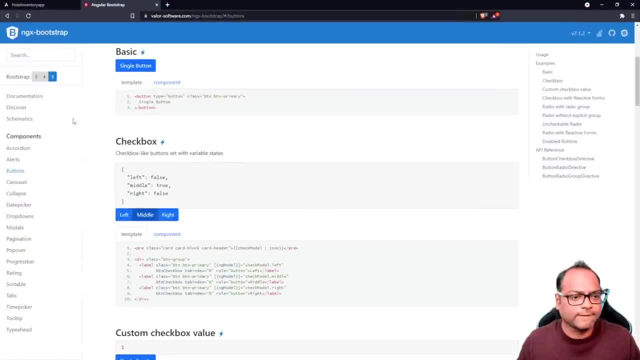 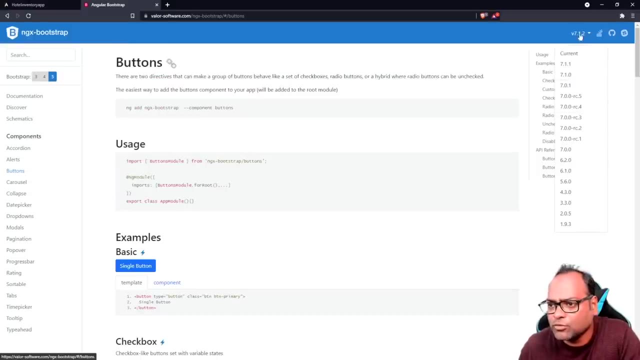 bootstrap 6.2.0 will be installed and bootstrap 6.2.0 will be installed and executed somehow. okay, uh, let's see what's wrong. so this ng uh njx bootstrap- the current. so this ng uh njx bootstrap- the current. so this ng uh njx bootstrap. the current version is 7.1.2. 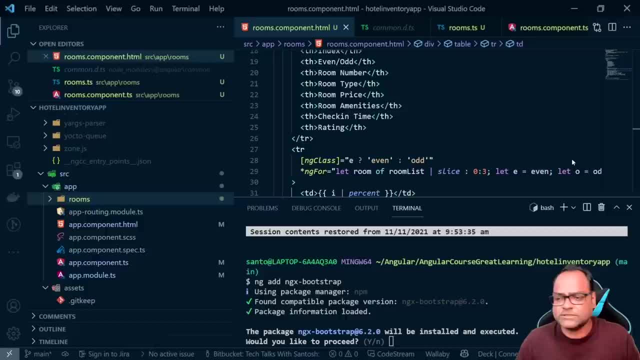 version is 7.1.2. version is 7.1.2, but it is saying for us the compatible. but it is saying for us the compatible, but it is saying for us the compatible version is 7, 6.2.0 version is 7, 6.2.0. 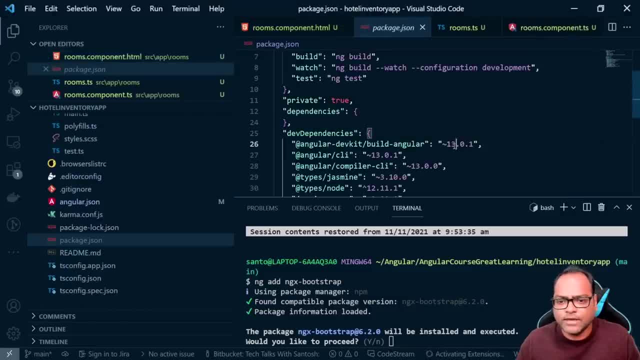 version is 7, 6.2.0, and we have angular 13, which is being used. we have angular 13, which is being used. we have angular 13, which is being used. so there is some problem with the. so there is some problem with the. 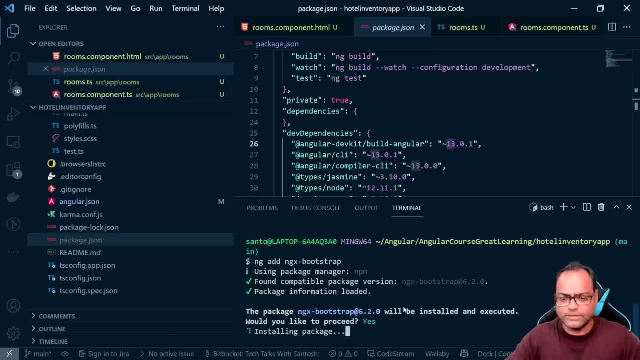 so there is some problem with the release. so let's use the uh latest release. so let's use the uh latest release. so let's use the uh latest version. whatever it is offering right version, whatever it is offering right version, whatever it is offering right now- 6.2.0 and. 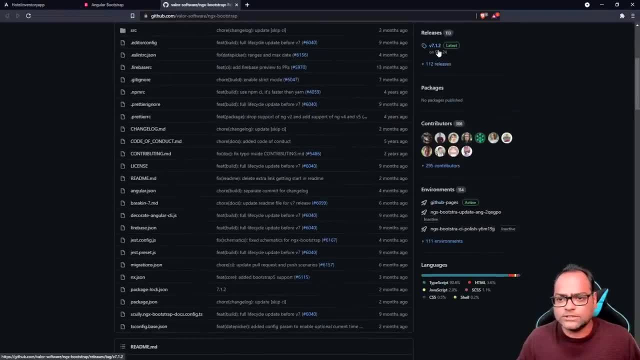 now 6.2.0, and now 6.2.0 and in a while i'll check what's wrong with. in a while i'll check what's wrong with. in a while i'll check what's wrong with this. so this, so this. so it is released on. 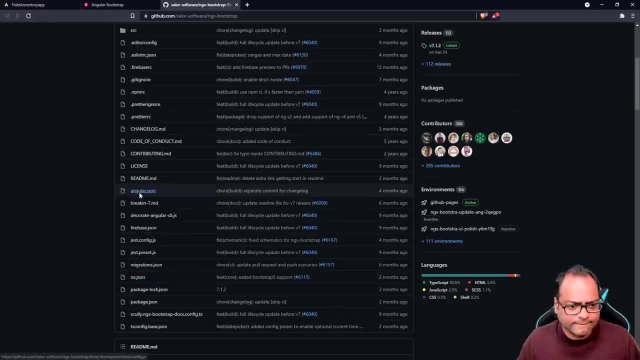 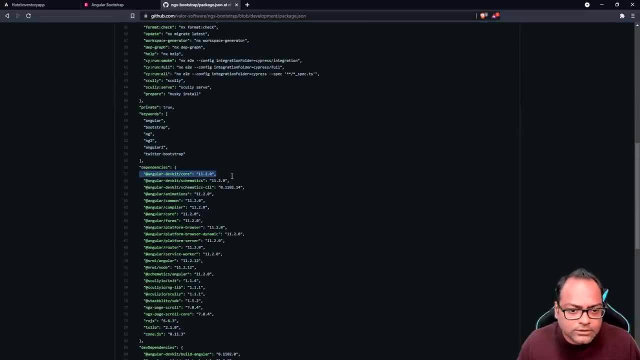 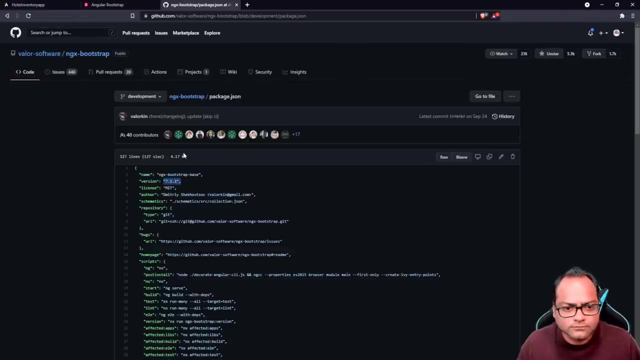 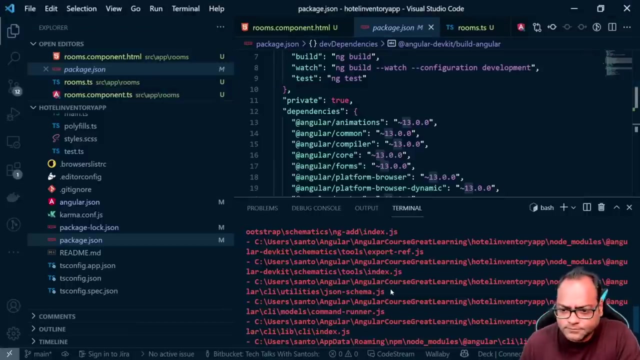 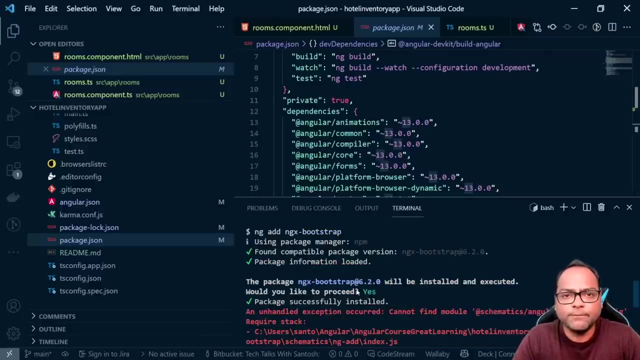 it is released on. it is released on september 24th, september 24th. cannot find schematic angular utility. cannot find schematic angular utility. cannot find schematic angular utility. config, config, config. okay, looks like this particular package. okay, looks like this particular package. okay. looks like this particular package is not compatible with angular 13 as of. 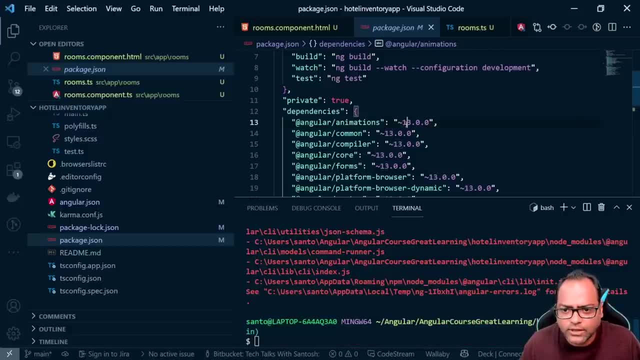 is not compatible with angular 13 as of is not compatible with angular 13 as of now. so that's that's the problem here now. so that's that's the problem here now. so that's that's the problem here, and and and what we can do. 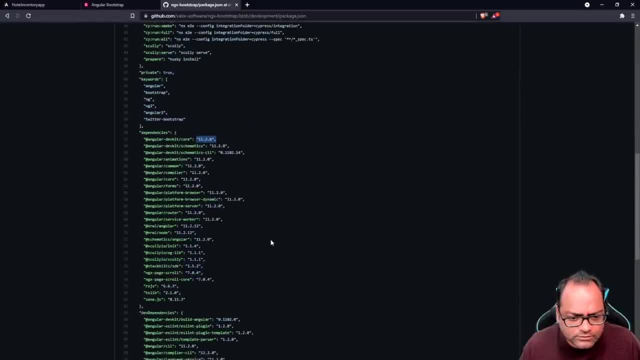 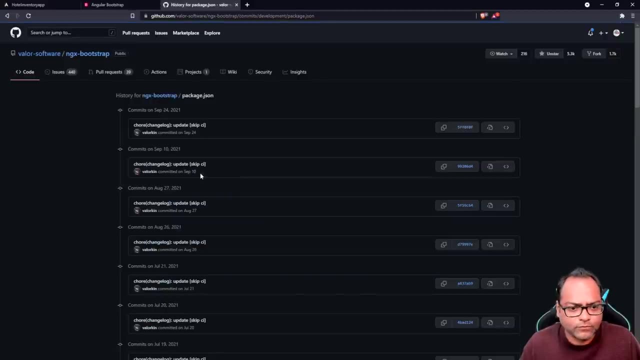 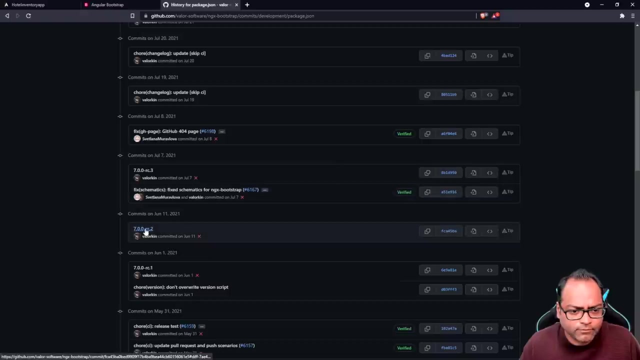 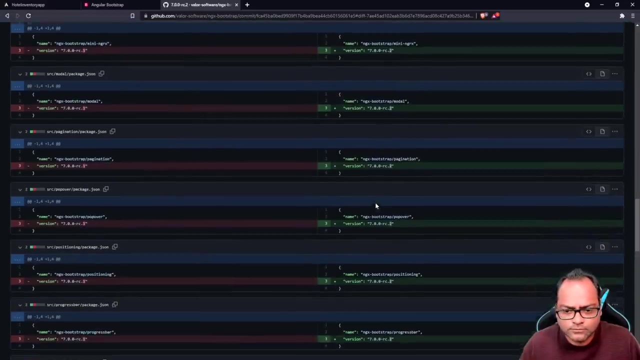 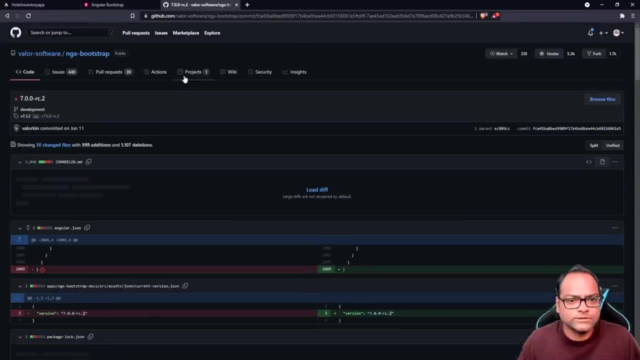 what we can do. what we can do, even they are not compatible with angular. even they are not compatible with angular. even they are not compatible with angular 12.. this is strange. okay, let's try with the uh. okay, let's try with the uh. okay, let's try with the uh. this version, which is 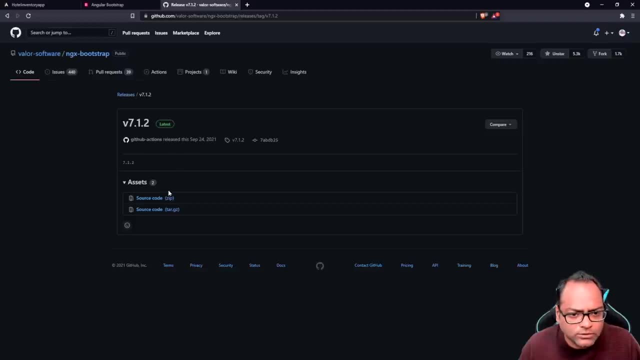 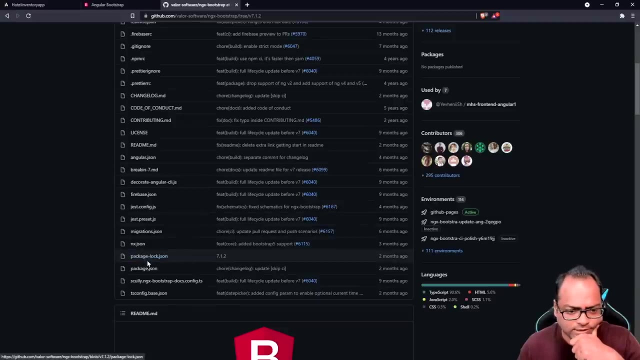 this version, which is this version, which is 7.1.2- okay, let's see 7.1.2. and then this one has: okay, let's see 7.1.2. and then this one has: okay, let's see 7.1.2. and then this one has packagejson which supports. 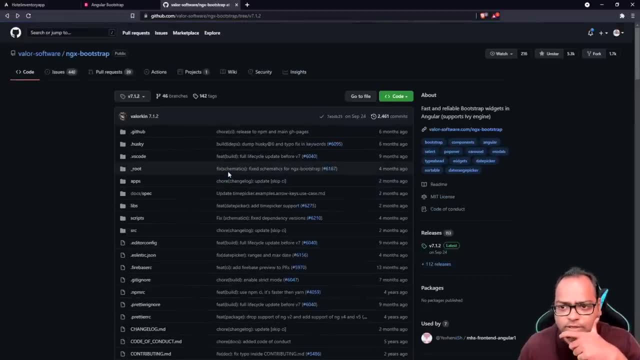 packagejson which supports packagejson which supports angular 11.. this is really strange, angular 11.. this is really strange, angular 11.. this is really strange because it should be, either because it should be, either because it should be either angular 12 or 13.. so let's. 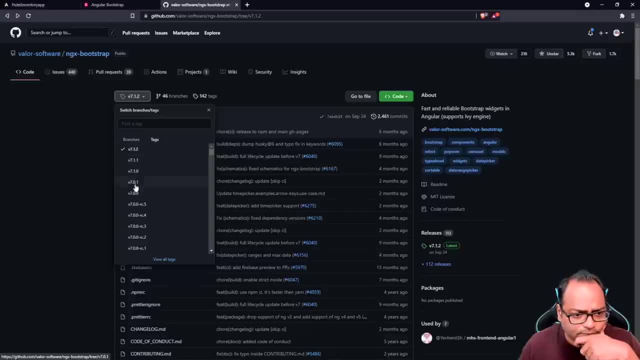 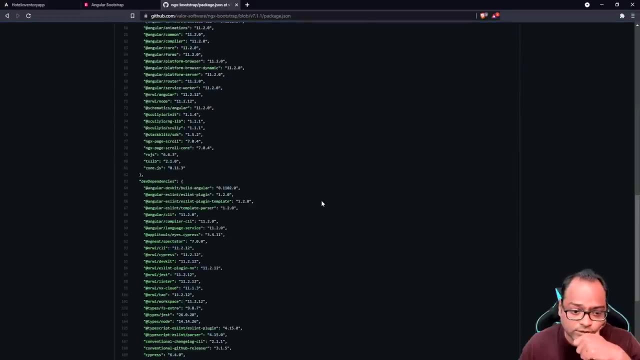 angular 12 or 13.. so let's angular 12 or 13.. so let's look for, look for, look for the tax, the tax, the tax 7.1.1. and this also uses angle 2, and this also uses angle 2. 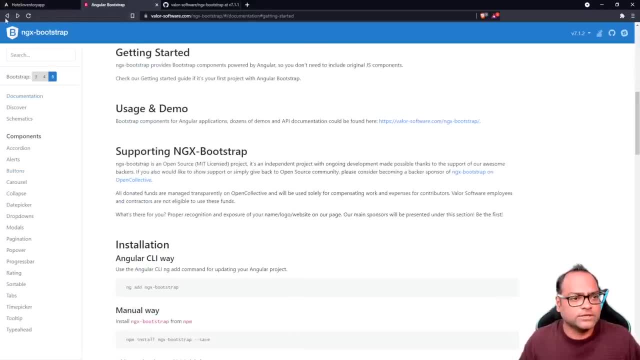 and this also uses angle 2. let's check if ng's. let's check if ng's. let's check if ng's. there is another package ng bootstrap. there is another package ng bootstrap. there is another package ng bootstrap. let's see if that supports it. let's see if that supports it. 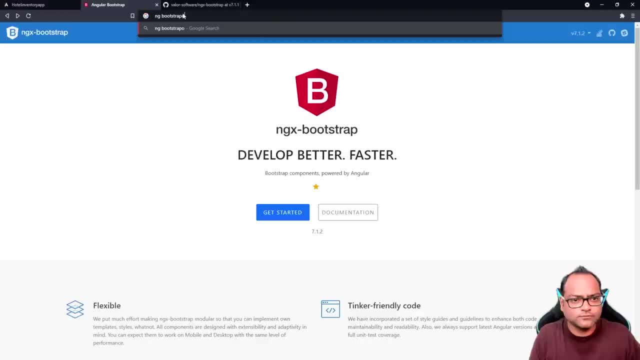 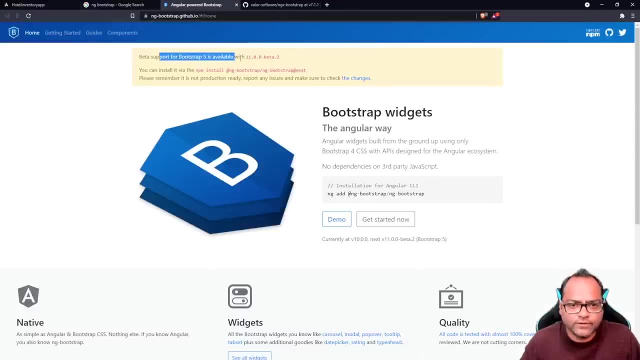 let's see if that supports it. ng book beta support for bootstrap 5 is available. beta support for bootstrap 5 is available. beta support for bootstrap 5 is available with angular 11, with with angular 11, with with angular 11, with 11.2. 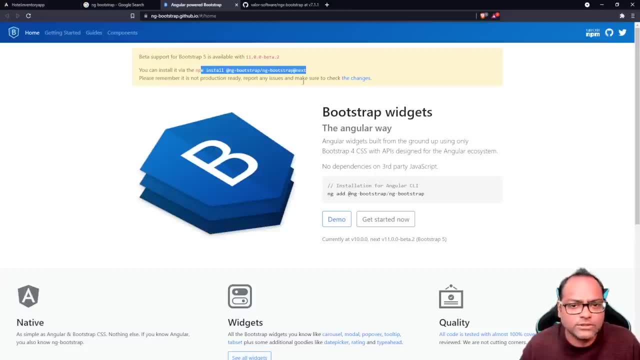 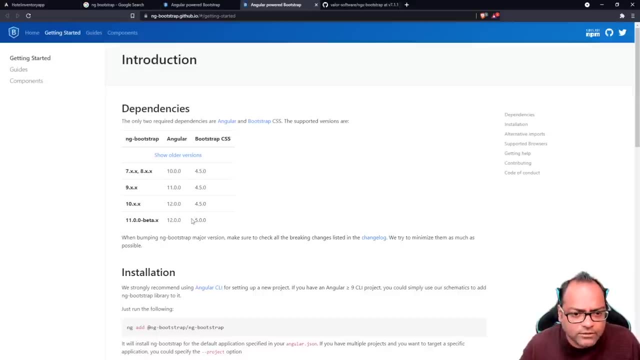 11.2, 11.2, 11.2, and this is the command. so let's see, and this is the command. so let's see, and this is the command. so let's see, uh, getting started, uh, getting started, uh, getting started. and this is for angular 12. 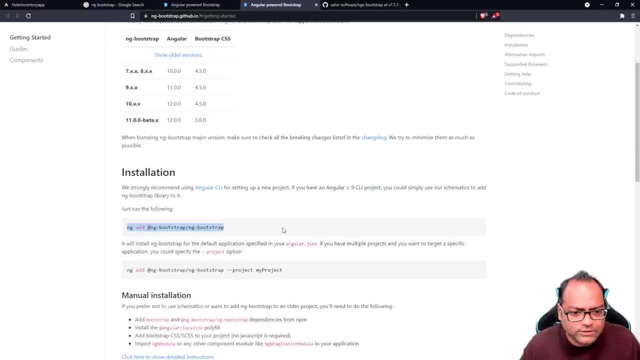 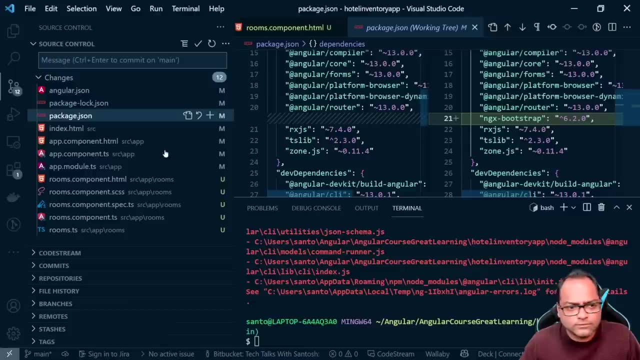 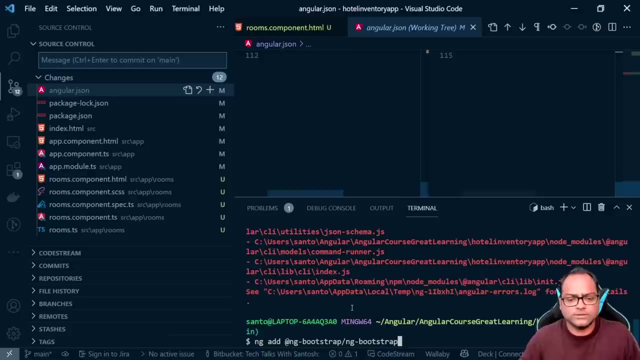 and this is for angular 12 and this is for angular 12: bootstrap, css5. bootstrap, css5, bootstrap, css5. let's try. let's try this one. and you bootstrap is added, and you bootstrap is added, and you bootstrap is added. okay, let's see if this works ng. 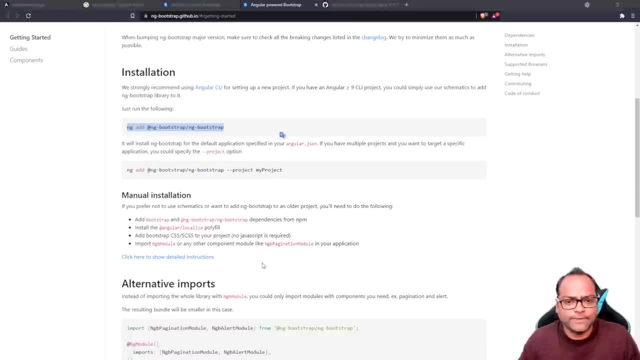 okay, let's see if this works ng. okay, let's see if this works ng. add ng bootstrap, so it also supports in case you have. so it also supports in case you have. so it also supports in case you have multiple projects, so you can pass multiple projects, so you can pass. 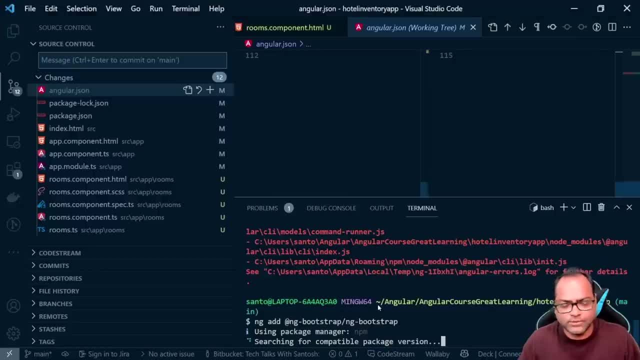 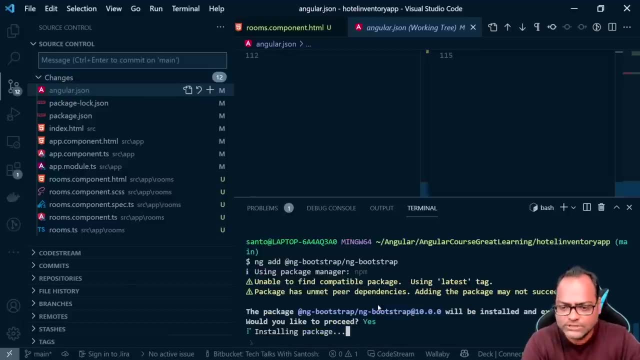 multiple projects so you can pass which project he wants to add this, which project he wants to add this, which project he wants to add this bootstrap library too. but let's see, okay, so it is saying bootstrap 10 will. okay, so it is saying bootstrap 10 will. 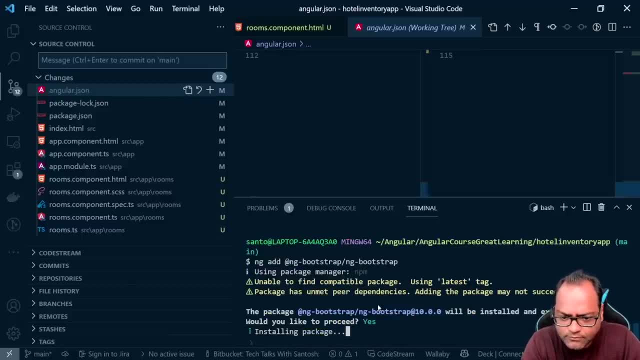 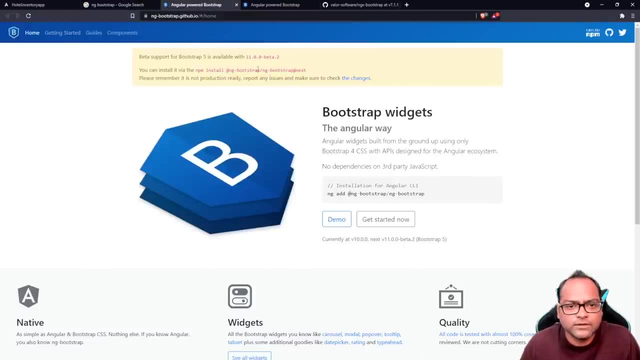 okay. so it is saying bootstrap 10 will be installed. okay, this is also just not working. so okay, this is also just not working. so okay, this is also just not working. so let's try, let's try, let's try with this one. so what i'm going to do? 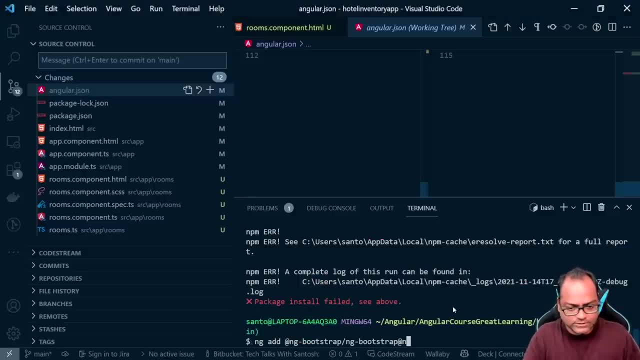 with this one, so what i'm going to do with this one, so what i'm going to do, is i'm going to do, is i'm going to do, is i'm going to do, and direct next. so, uh, remember as of today, not all the. so, uh, remember as of today, not all the. 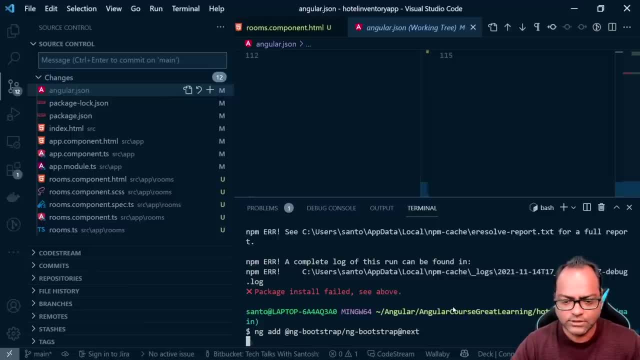 so, uh, remember, as of today, not all the libraries are compatible with angular libraries are compatible with angular libraries are compatible with angular 13, and that's what 13, and that's what 13, and that's what. uh, we are, that's what the issue which 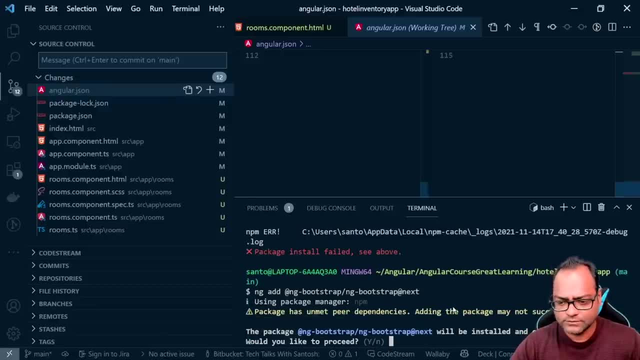 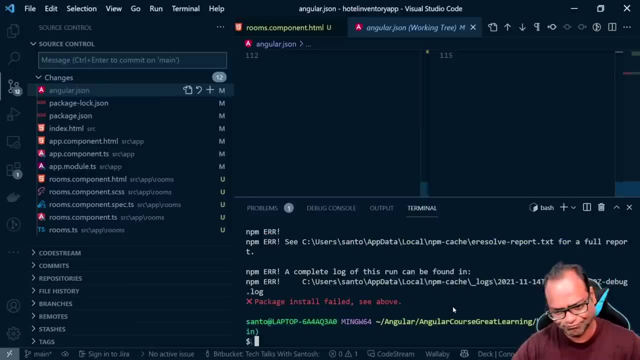 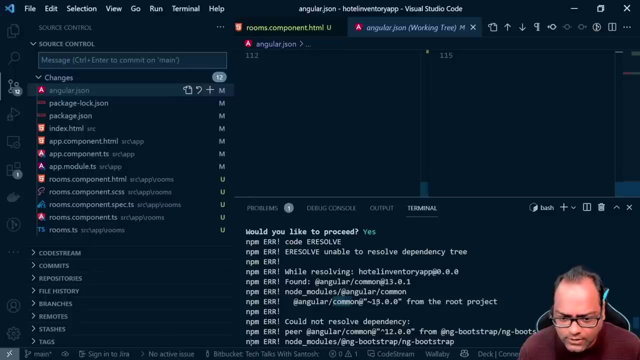 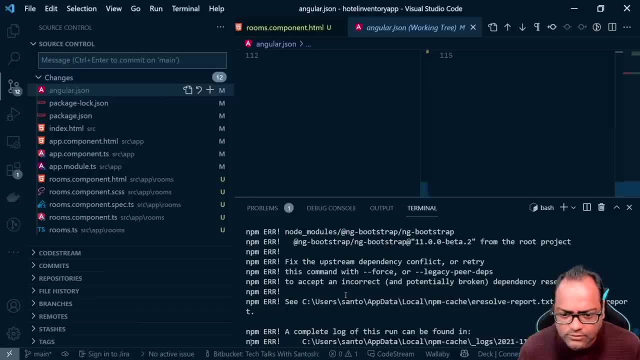 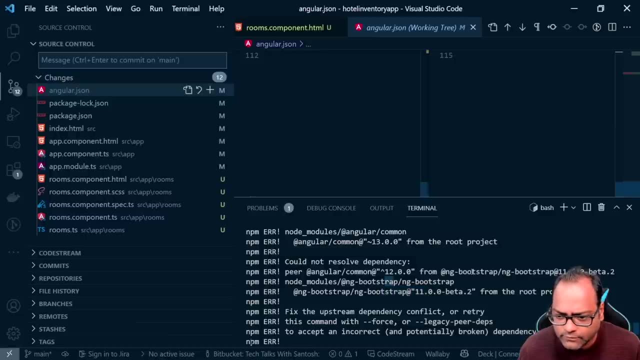 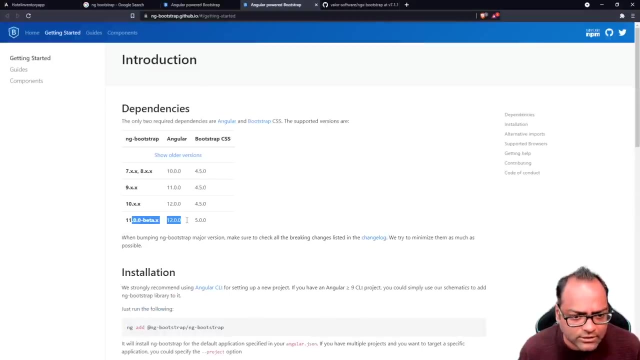 angular 13 from boot project found common 13.0.1. angular common 12. okay so even they are not compatible. okay so, even they are not compatible. okay so, even they are not compatible with angular 13, because they are saying with angular 13, because they are saying: 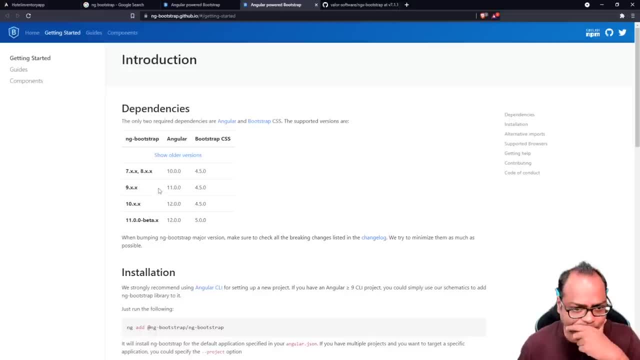 with angular 13 because they are saying, okay, this is for angular 12. okay, this is for angular 12. okay, this is for angular 12, okay, okay, okay, this is for angular 12. okay, let's see if we have any other way. let's see if we have any other way. 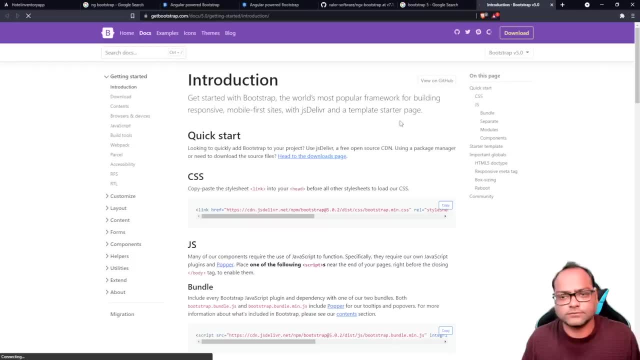 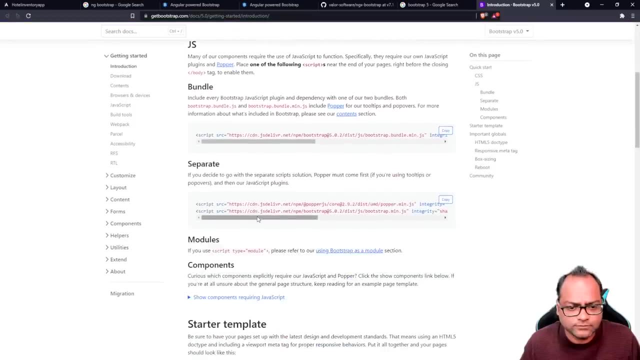 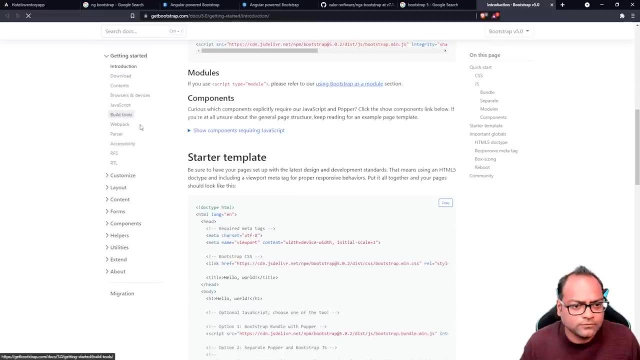 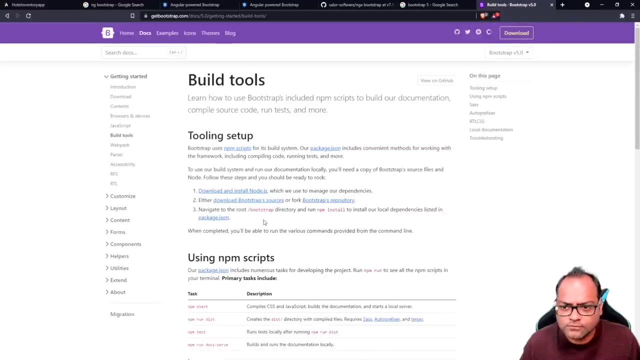 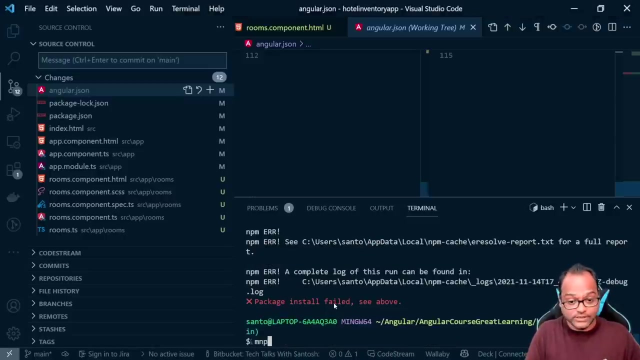 let's see if we have any other way. start by start by, start by. let's start from here. let's start from here: 5.0 okay, so it is available. 5.0 okay, so it is available. 5.0 okay, so it is available. let's try to install bootstrap directly. 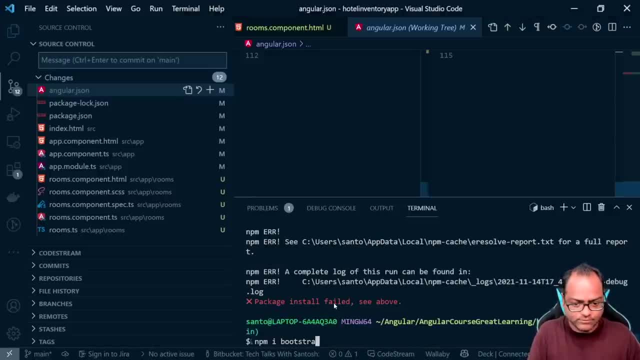 let's try to install bootstrap directly. let's try to install bootstrap directly, and then we'll see and then install, and then we'll see, and then install, and then we'll see and then install: bootstrap, bootstrap, bootstrap. so, uh, if you are not aware, bootstrap 5. 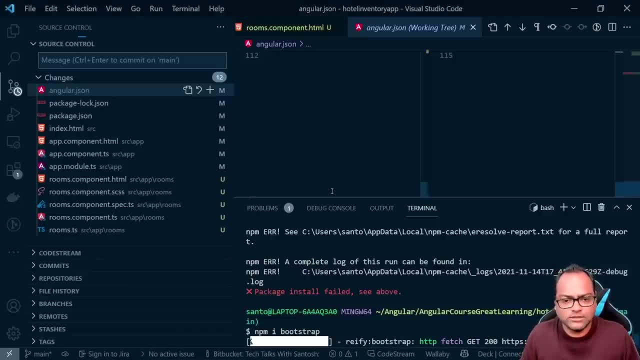 so, uh, if you are not aware, bootstrap 5: so uh, if you are not aware, bootstrap 5 has actually dropped the support for, has actually dropped the support for, has actually dropped the support for. either so that's either. so that's either. so that's. that's one thing which they have done. 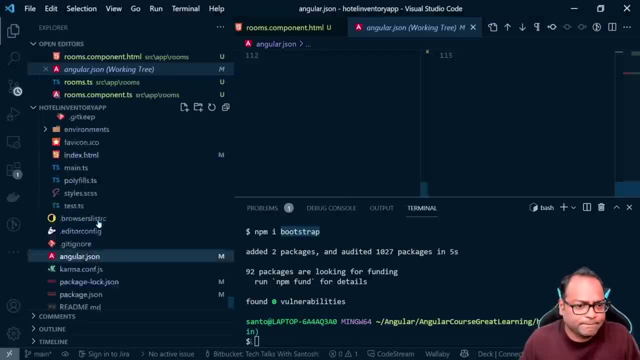 that's one thing which they have done. that's one thing which they have done. so bootstrap is installed. now let's see. so you can verify it from node modules. so you can verify it from node modules. so you can verify it from node modules folder, which we have available here. 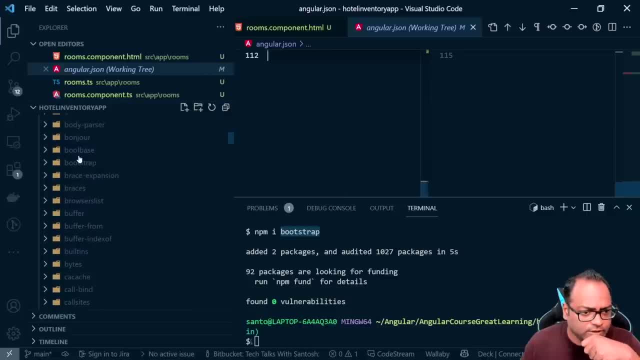 folder which we have available here, folder which we have available here. and let's go to a b bootstrap and let's go to a b bootstrap and let's go to a b bootstrap. so distributable js and sorry css. and so distributable js and sorry css. and 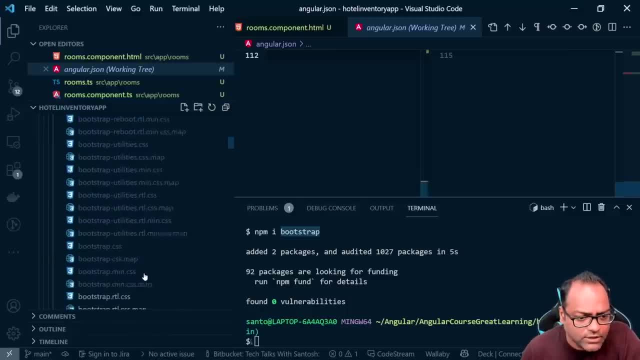 so distributable js and sorry, css. and okay, this is okay. this is okay. this is all bootstrap css files which is available, all bootstrap css files which is available. all bootstrap css files which is available. we want to use bootstrapmeancss. we want to use bootstrapmeancss. 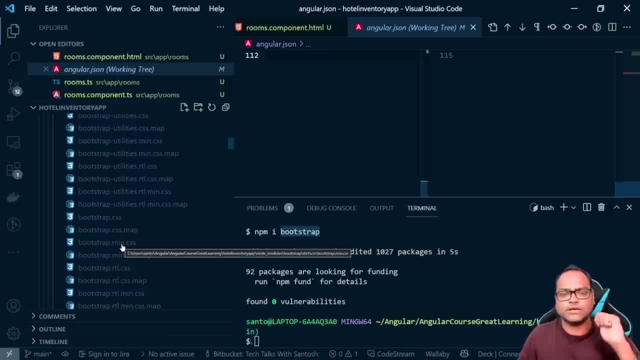 we want to use bootstrapmeancss. this is what we are going to use, and this is what we are going to use, and this is what we are going to use. and there are multiple ways. there are. there are multiple ways there are. there are multiple ways. there are multiple ways you can do it. 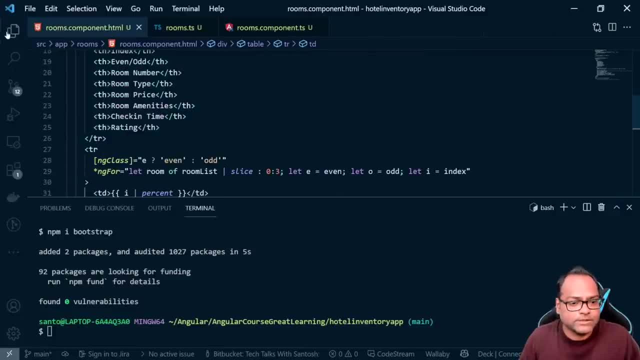 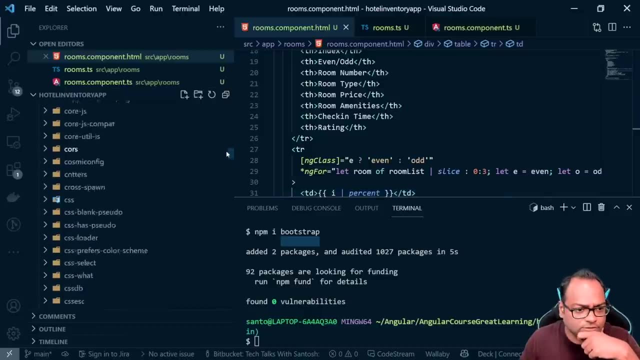 multiple ways you can do it. multiple ways you can do it. let's see, let's see, let's see, start to configure it. so start to configure it, so start to configure it. so, okay, i have to, okay, i have to, okay, i have to. i want you to copy the path, actually so 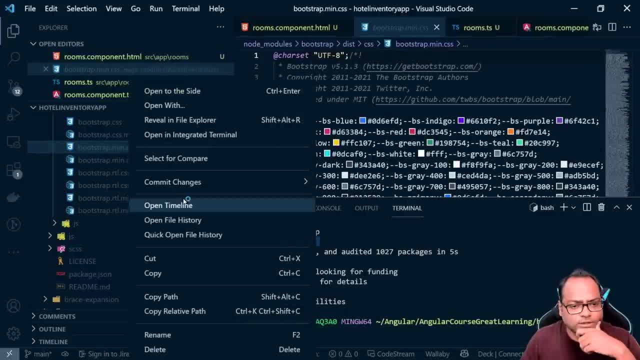 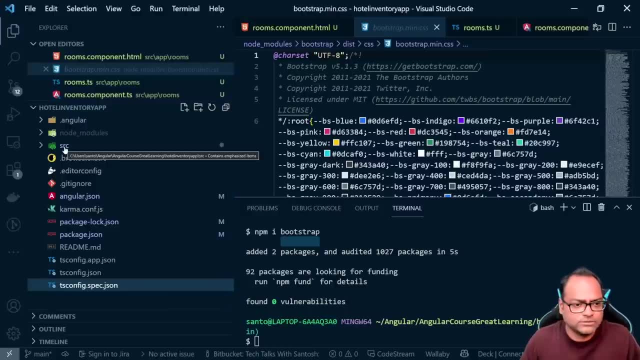 i want you to copy the path actually. so i want you to copy the path actually. so here bootstrap meaning dot css. here bootstrap meaning dot css. here bootstrap meaning dot css. i'll copy, i'll copy, i'll copy relative path and and and i'll show you both ways. 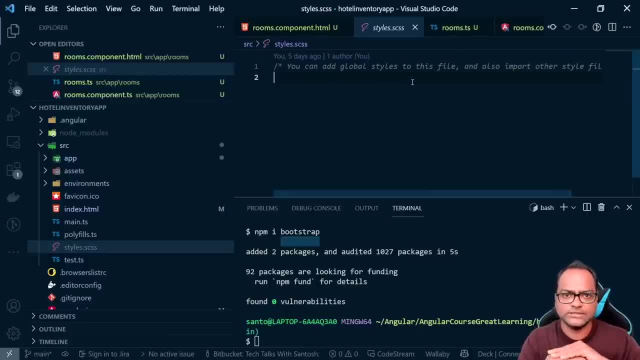 first, first, first, first, first, first, first way is: you can actually add this way, is you can actually add this way, is you can actually add this uh css into your global global styling, uh css into your global global styling, uh css into your global global styling? how you can do that so you can use import. 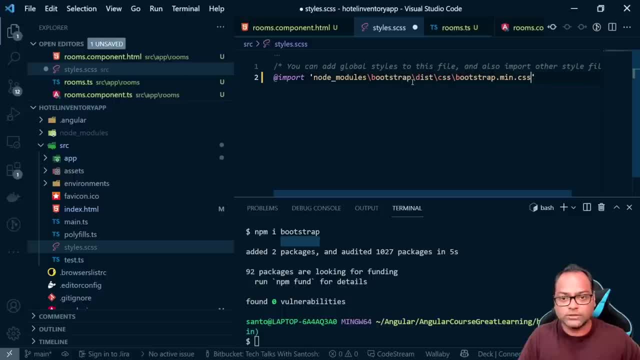 how you can do that so you can use import. how you can do that so you can use import, sorry, add the right import. and then you, sorry, add the right import, and then you, sorry, add the right import, and then you can do, can do, can do this. you don't have to actually give. 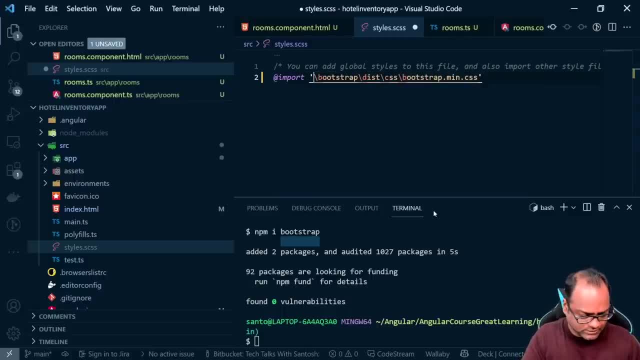 this. you don't have to actually give this, you don't have to actually give path like this. you can just say path like this. you can just say path like this. you can just say: uh, uh, uh, build this this one, build this this one, build this, this one and, of course, change. 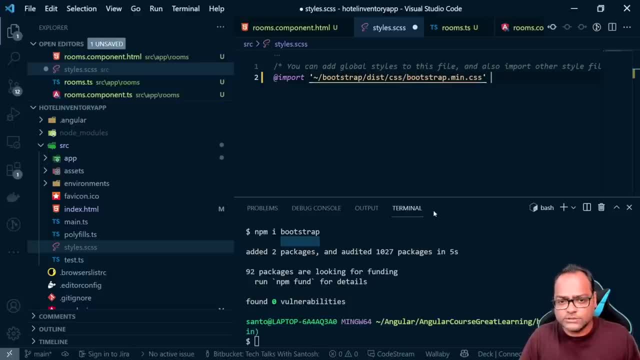 and of course change, and of course change pst css, pst css, pst css, window css and window css and window css, and let's try to see, if let's try to see, if let's try to see if this one works so, and then we'll show this one works so and then we'll show. 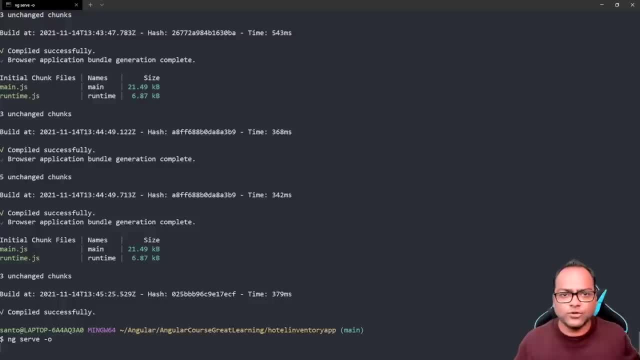 this one works so, and then we'll show you another bit which is uh, not you. another bit which is uh, not you. another bit which is uh, not adding to your global style css, but in adding to your global style css, but in adding to your global style css, but in another way. 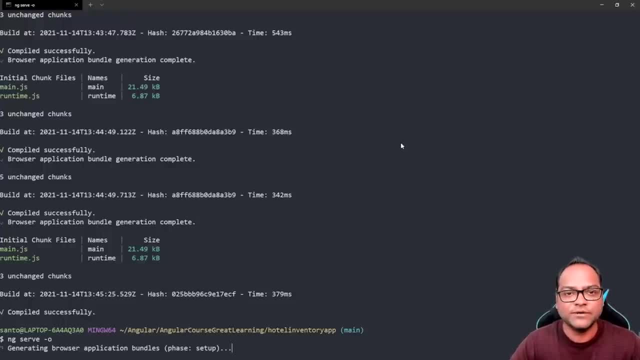 we'll be able to see the changes. because we'll be able to see the changes, because we'll be able to see the changes because, of course, styling of your page will, of course, styling of your page will, of course, styling of your page will change because of the font which is. 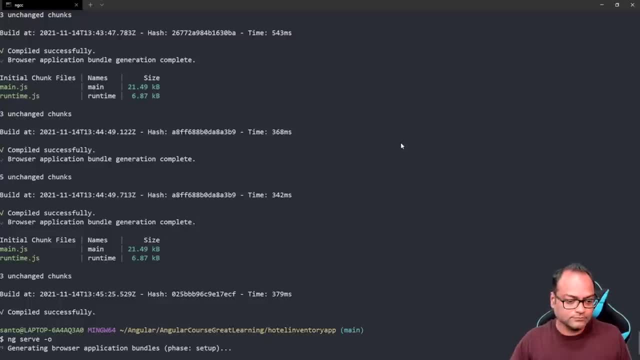 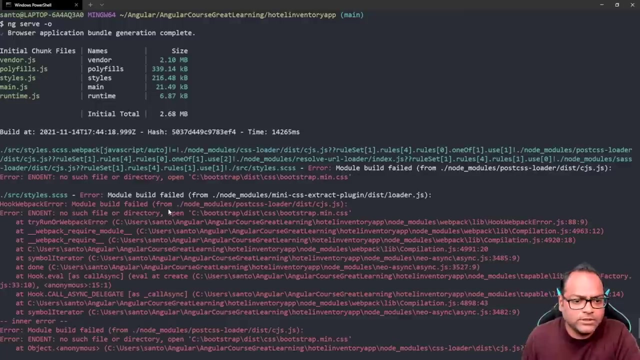 change because of the font which is change because of the font which is used by bootstrap. okay, let's. there's some error. no such file directory. there's some error, no such file directory. there's some error, no such file directory. open bootstrap dst. okay. open bootstrap dst- okay. 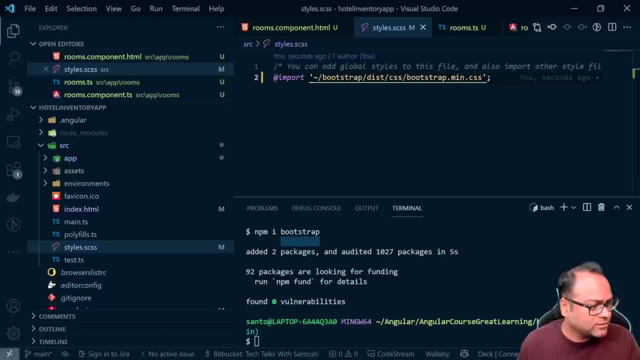 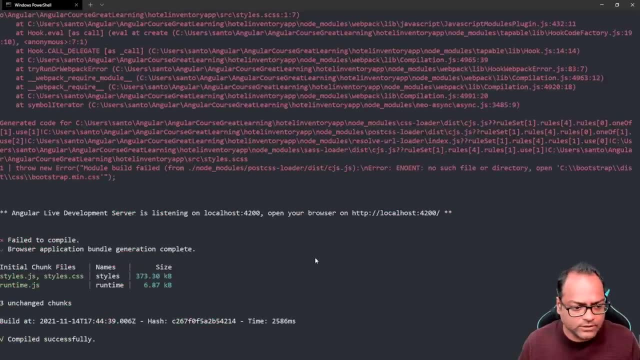 open bootstrap dst. okay, what is? what is what is wrong here? probably, let's remove this, let's remove this, let's remove this, and let's see our build, and let's see our build and let's see our build. okay, now it is compiled successfully. so, okay, now it is compiled successfully. so. 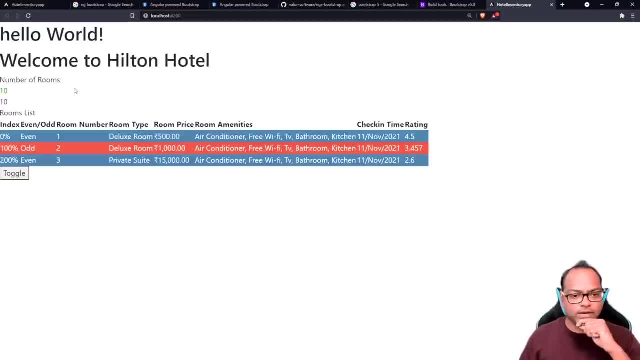 okay, now it is compiled successfully. so let's, let's, let's see. okay, so you can see. uh, i think you see. okay, so you can see. uh, i think you see. okay, so you can see. uh, i think you might have seen this page, you can see. 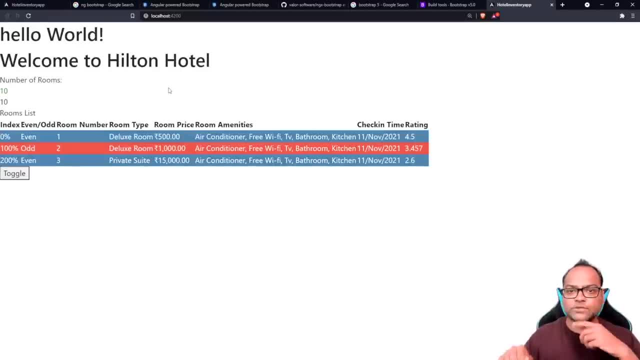 might have seen this page you can see. might have seen this page. you can see. this page and this page, this page and this page, this page and this page. so this one has bootstrap 5, which is so. this one has bootstrap 5, which is so. this one has bootstrap 5, which is installed and now applicable to. 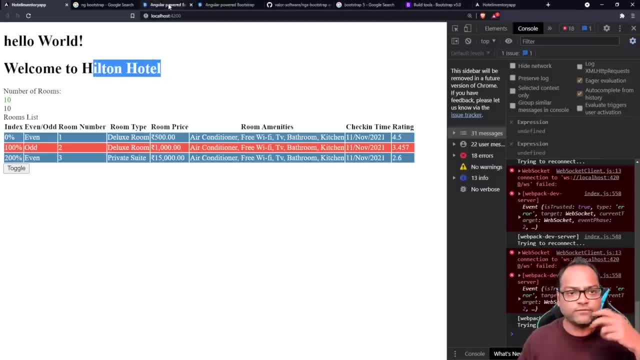 installed and now applicable to. installed and now applicable to your application. this doesn't have any your application. this doesn't have any your application. this doesn't have any css. so this is how you can verify if css. so this is how you can verify if css. so this is how you can verify if uh bootstrap is added to your application. 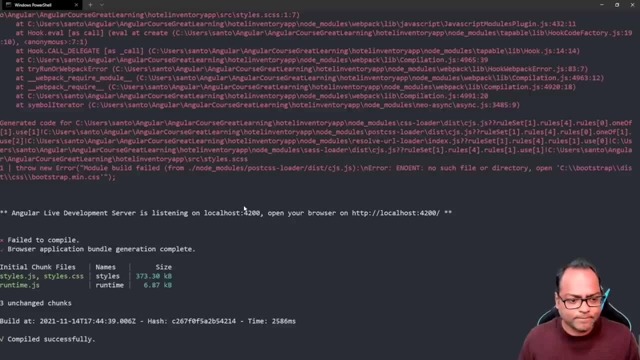 uh, bootstrap is added to your application. uh, bootstrap is added to your application or not, or not, or not, so, so, so, let me show you another way to add, let me show you another way to add, let me show you another way to add bootstrap or any other css. so it's, it's. 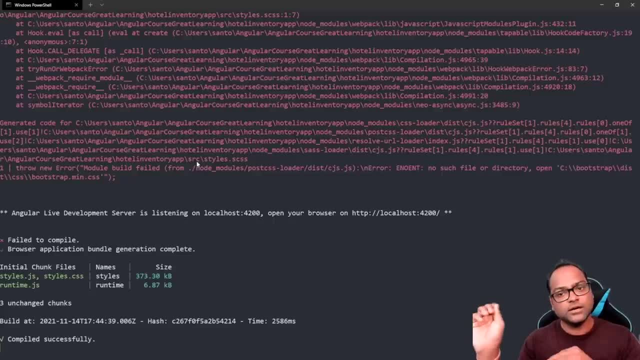 bootstrap or any other css. so it's. it's bootstrap or any other css, so it's. it's something which you can do with any css, something which you can do with any css, something which you can do with any css, any, any, any css which you have installed using npm. 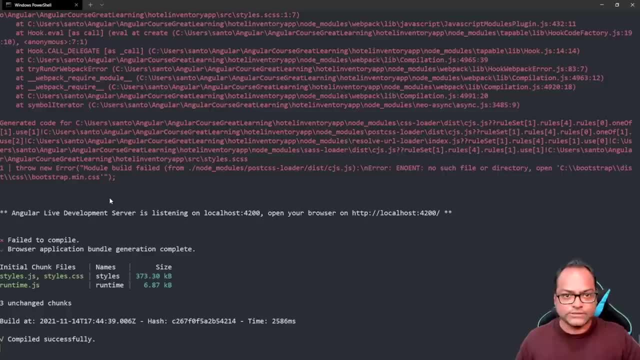 css, which you have installed using npm. css, which you have installed using npm, so it's not only for bootstrap. so, so it's not only for bootstrap. so so it's not only for bootstrap. so this was the first way where you can. this was the first way where you can. 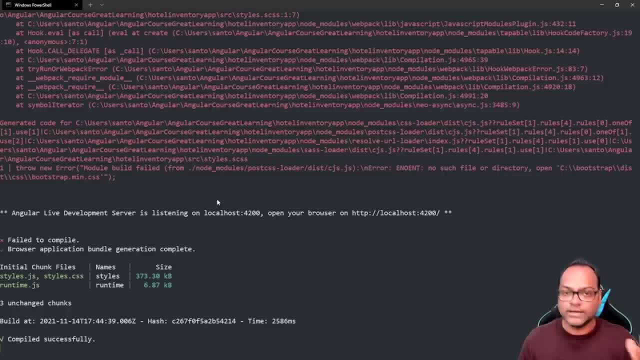 this was the first way where you can actually go ahead and add it into style, actually go ahead and add it into style, actually go ahead and add it into stylecss, css, css or css, whatever, or css, whatever or css, whatever type which you are using. 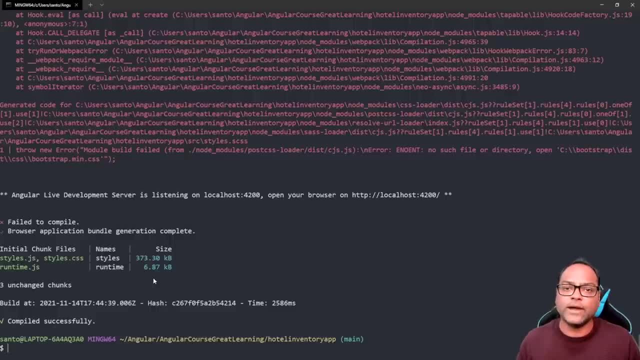 type which you are using, type which you are using. so let's stop the server because in so let's stop the server because in. so let's stop the server because in another way, we are going to add this. another way, we are going to add this, another way we are going to add this into our. 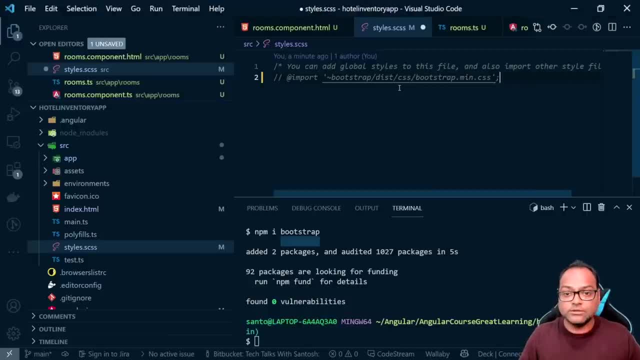 into our, into our angularjson, so i'll comment this out. so we don't have, so i'll comment this out. so we don't have, so i'll comment this out. so we don't have this css available here, this css available here, this css available here, and i can go to angularjson, angularjson. 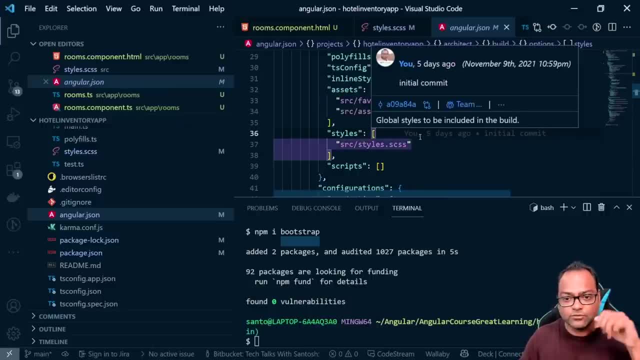 and i can go to angularjson, angularjson, and i can go to angularjson. angularjson has many properties. there is one has many properties, there is one has many properties. there is one property called styles, property called styles, property called styles, and i can go here and 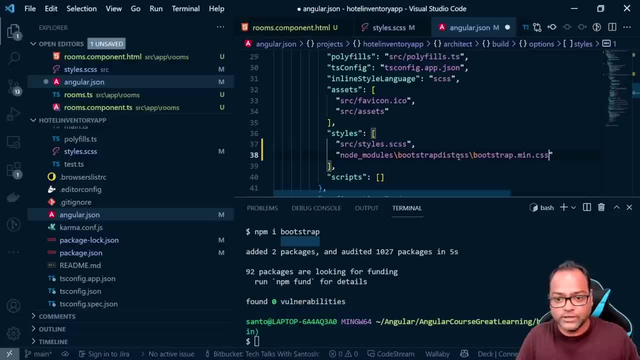 and i can go here, and, and i can go here and i can apply: uh, just it's an array, i can apply. uh, just it's an array, i can apply. uh, just it's an array, remember, and i can just go ahead and add. remember, and i can just go ahead and add. 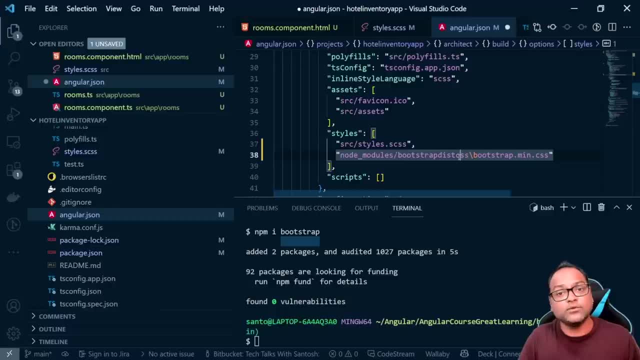 remember and i can just go ahead and add this path, this path, this path, okay, bootstrap, okay, bootstrap, okay, bootstrap based css, based css based css and bootstrap maincss and bootstrap maincss and bootstrap maincss and and and. if i'm not wrong, bootstrap also gives. if i'm not wrong, bootstrap also gives. 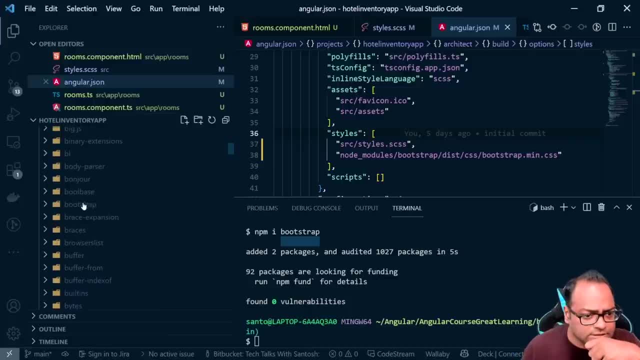 if i'm not wrong, bootstrap also gives you you you sas file. you can also use that. let's see sas file. you can also use that. let's see sas file. you can also use that. let's see tsd css, and i think you will. 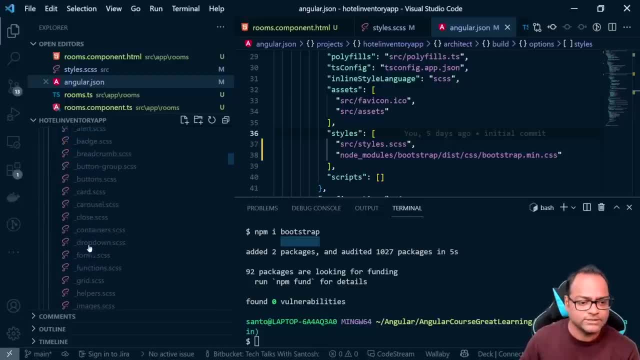 and i think you will, and i think you will here it is so, in case you want to add here it is so, in case you want to add, here it is so in case you want to add or use sas files. this is: or use sas files. this is: 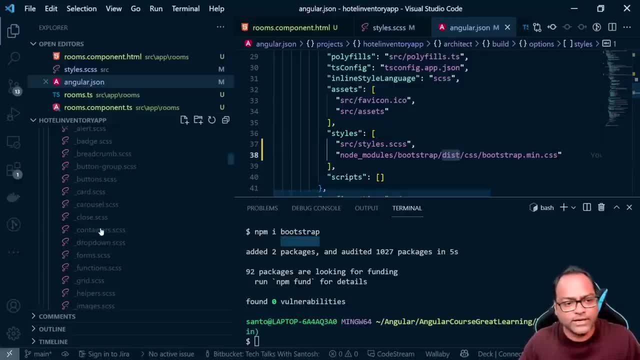 or use sas files. this is, sas files are available as well. so rather, sas files are available as well, so rather, sas files are available as well. so, rather than actually taking the path from, than actually taking the path from, than actually taking the path from, least you will be taking it from scss. 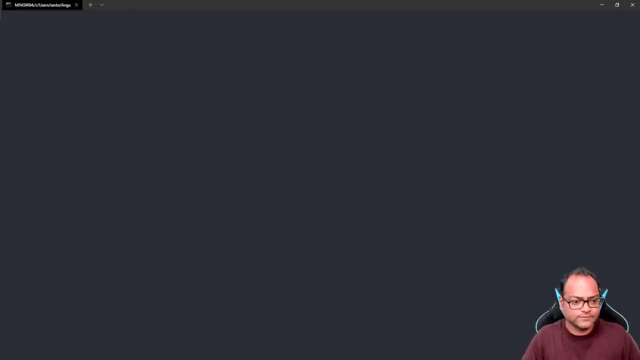 least you will be taking it from scss, least you will be taking it from scss folder. that's, that's the difference folder. that's, that's the difference folder. that's, that's the difference. and now let's run it again. and now let's run it again. 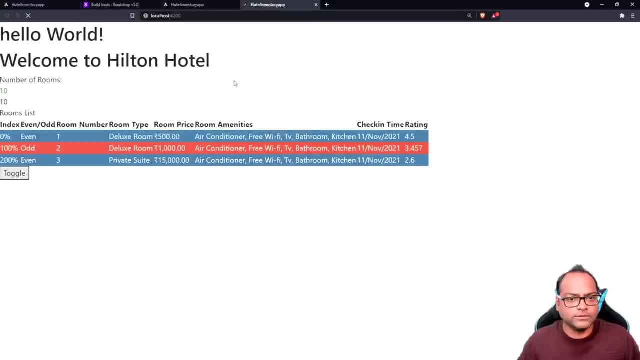 and now let's run it again, and done and and done and and done, and you can see- uh, of course you can see, you can see. uh, of course you can see, you can see. uh, of course you can see the difference, right, so you have, this is. 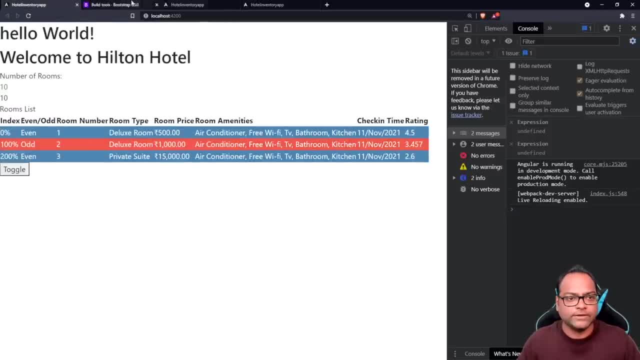 the difference, right, so you have. this is the difference, right, so you have. this is with bootstrap 5, and this is without any with bootstrap 5, and this is without any with bootstrap 5, and this is without any style, with being added to our style, with being added to our. 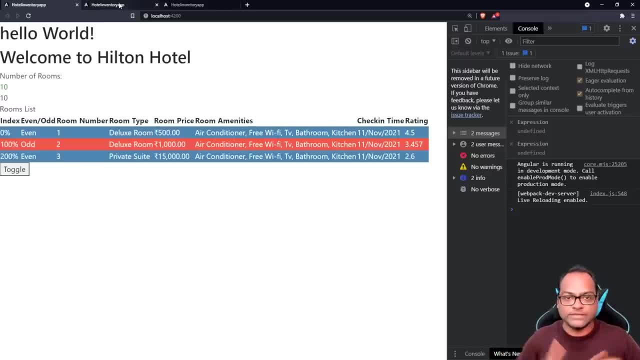 style with being added to our application. so right now, of course, as of application. so right now, of course, as of application. so right now, of course, as of today ng bootstrap ng bootstrap, do. today ng bootstrap ng bootstrap, do today ng bootstrap ng bootstrap, do. both are not supported with angular 13, but. both are not supported with angular 13, but both are not supported with angular 13, but in future they will, so, in future they will, so, in future they will so, uh, the only difference would be: you have uh. the only difference would be: you have uh. the only difference would be: you have to run that ng add command. 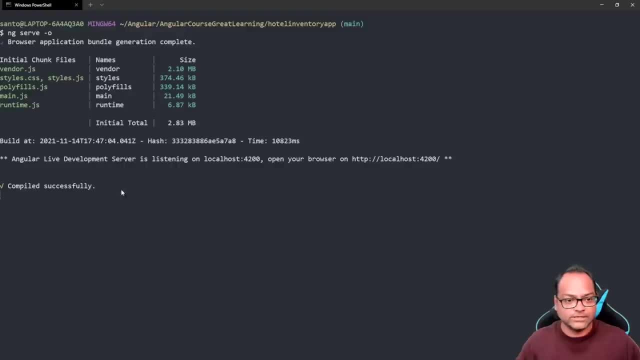 to run that ng add command, to run that ng add command, and you don't have to, and you don't have to, and you don't have to set this con, this uh changes which we set, this con, this uh changes which we set this con. this uh changes which we did right now, right so. 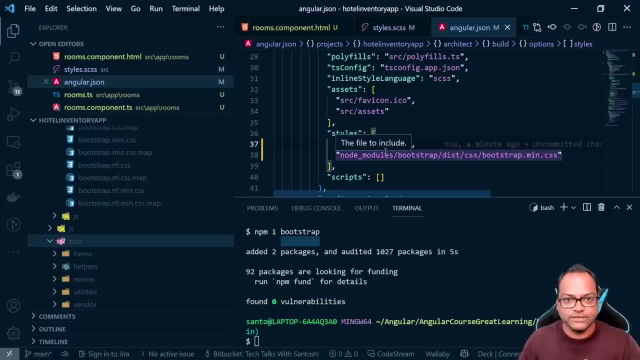 did right now, right. so, did right now, right. so we added this to styles uh array you. we added this to styles uh array you. we added this to styles uh array. you don't have to do this manually. don't have to do this manually. don't have to do this manually. that will be taken care by ng. add command. 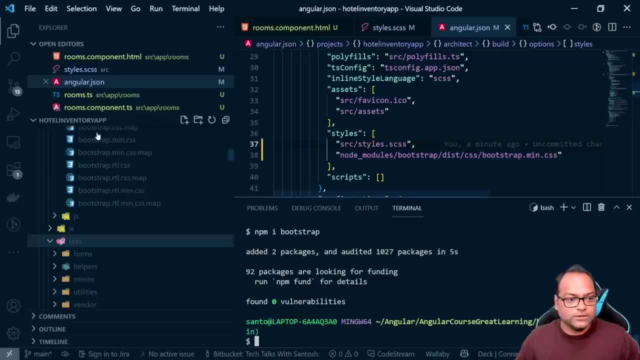 that will be taken care by ng add command. that will be taken care by ng add command, which we used previously. so now we know how to use uh this. so now we know how to use uh this. so now we know how to use uh this ss. so let's try to actually apply some. 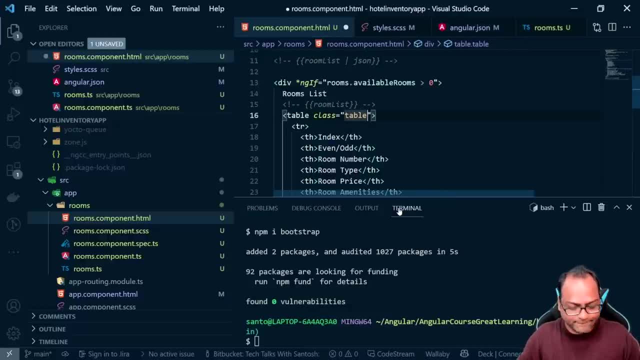 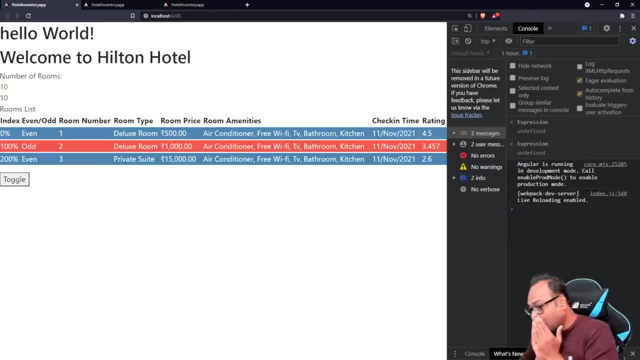 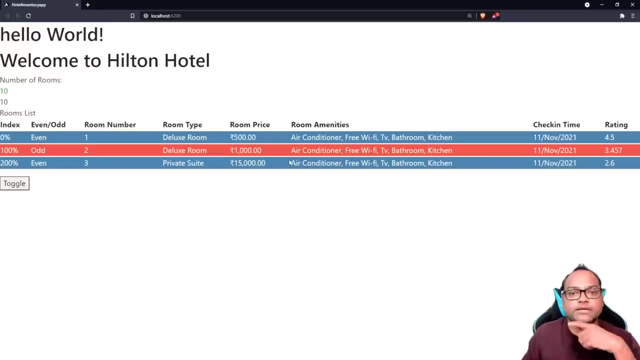 ss. so let's try to actually apply some ss. so let's try to actually apply some css here, css here, css here. class table. let me close this now. uh, you can see this. let me close this now. uh, you can see this. let me close this now. uh, you can see, this table is uh. 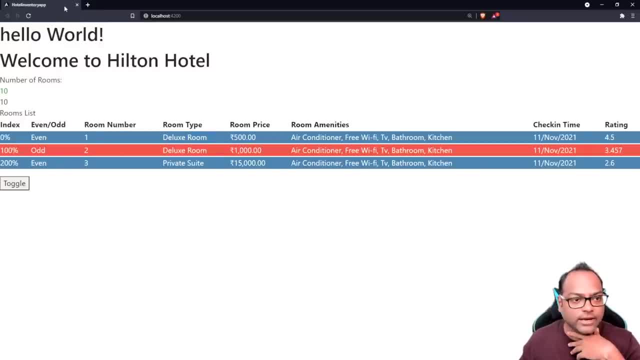 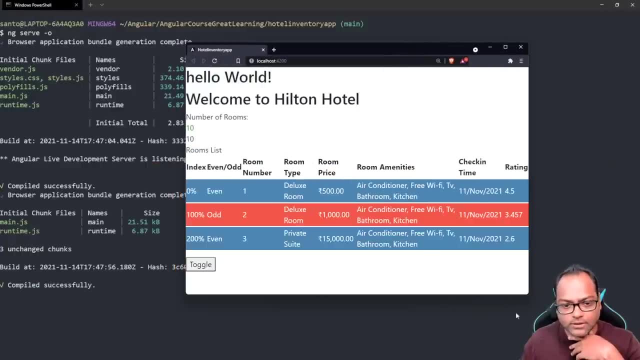 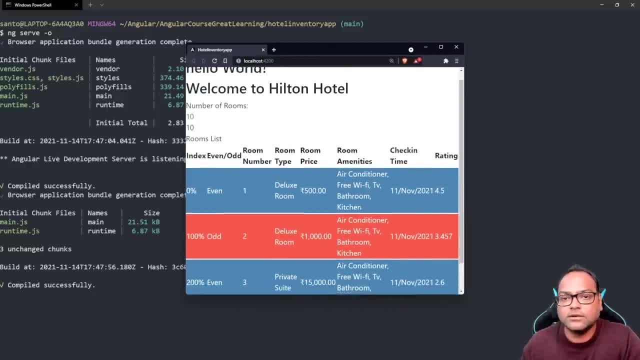 right, so we have. you can see right, so we have. you can see right, so we have. you can see, as we added bootstrap, now our application, as we added bootstrap, now our application, as we added bootstrap, now our application is responsive, so it is is responsive, so it is. 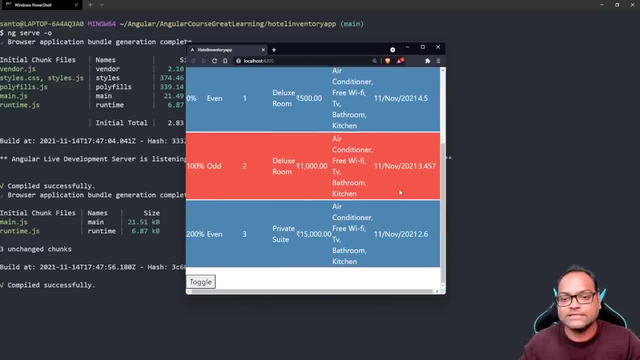 is responsive, so it is changing the width of your table based on changing the width of your table, based on changing the width of your table based on your screen size, your screen size, your screen size. so you don't have to do that manually. so you don't have to do that manually. 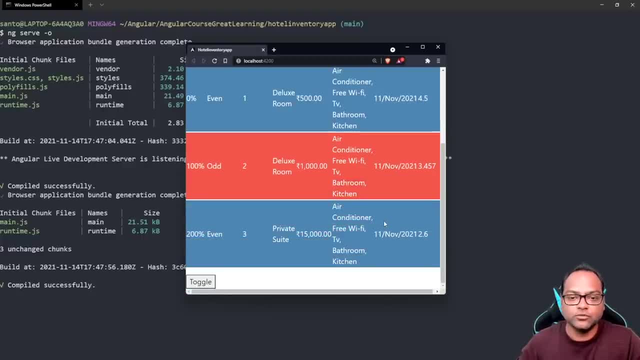 so you don't have to do that manually anymore. i mean you don't have to add anymore. i mean you don't have to add anymore. i mean you don't have to add extra styles, extra styles, extra styles. uh, to make your application responsive, uh, to make your application responsive. 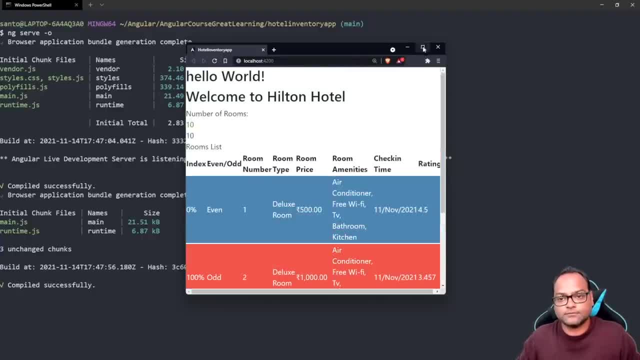 uh, to make your application responsive. bootstrap will take care of it. bootstrap will take care of it. bootstrap will take care of it for you in this video we are going to talk about. in this video we are going to talk about. in this video we are going to talk about, life cycle looks. 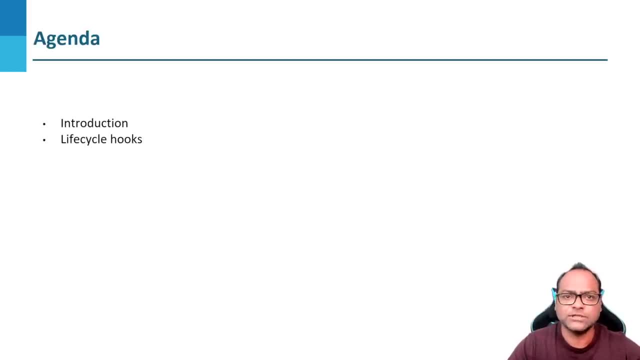 life cycle looks. life cycle looks, so we'll talk about what life cycle looks. so we'll talk about what life cycle looks, so we'll talk about what life cycle looks is, and then what are the different is, and then what are the different is, and then what are the different life cycle looks which exist. 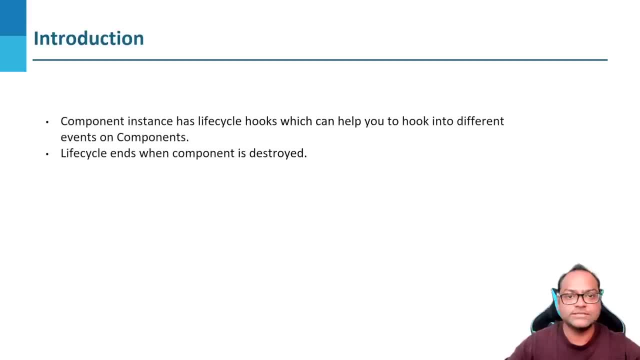 life cycle looks which exist. life cycle looks which exist for uh your components, for uh, your components for uh, your components. so let's see what is component uh, or so let's see what is component, uh, or so let's see what is component uh, or life cycle look. is so in angular, what? life cycle look is so in angular. what life cycle look is so in angular? what we are going to create is we are going to. we are going to create is we are going to. we are going to create is we are going to, of course, go ahead and create a lot of. 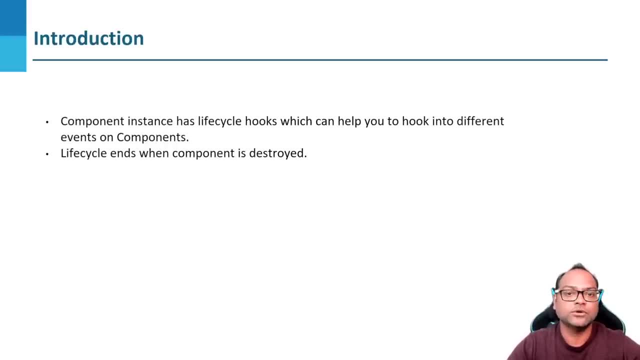 of course, go ahead and create a lot of. of course, go ahead and create a lot of components, components, components. now, all component needs to go through now. all component needs to go through now, all component needs to go through some life cycle hooks, some life cycle hooks, some life cycle hooks, or you can say, some events which it 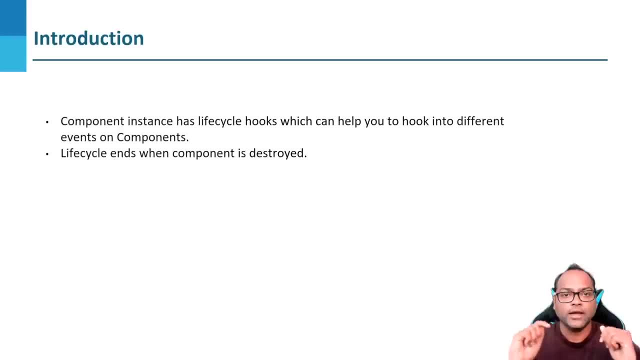 or you can say some events which it, or you can say some events which it needs to go through. this will happen this entire. this will happen this entire. this will happen, this entire events, or you can say hooks, will happen. events, or you can say hooks will happen. 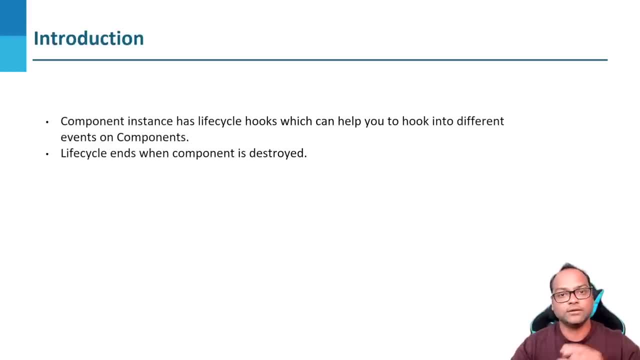 events, or you can say hooks, will happen for each and every component, for each and every component, for each and every component. so in other technologies also, in other so, in other technologies also, in other so in other technologies also, in other frameworks also. you have, frameworks also, you have. 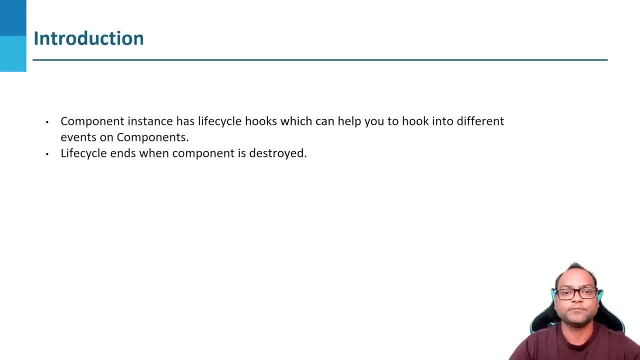 frameworks. also, you have the concept of hooks, and same applies to the concept of hooks and same applies to the concept of hooks and same applies to angular, angular, angular in dotnet. in case you are coming from in dotnet, in case you are coming from in dotnet, in case you are coming from dotnet. 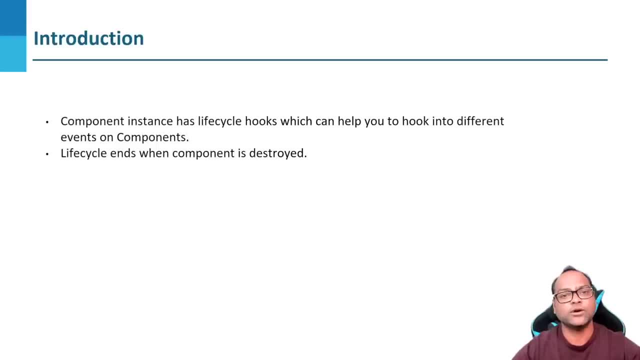 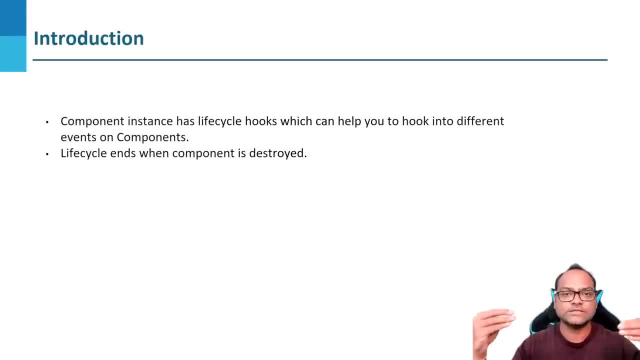 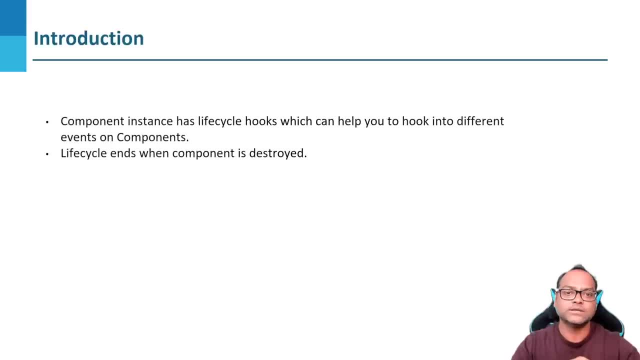 component of a com. sorry if you talk component of a com, sorry if you talk about event or life cycle. hook for a about event or life cycle. hook for a about event or life cycle. hook for a component, component, component. so somewhere it starts creating a new. so somewhere it starts creating a new. 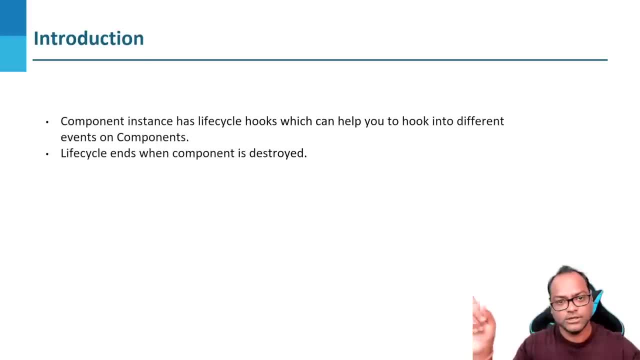 so somewhere it starts creating a new instance for component, and at the end it instance for component, and at the end it instance for component, and at the end it will be destroyed, so will be destroyed, so will be destroyed. so, from start, for, from creating an instance, from start for from creating an instance. 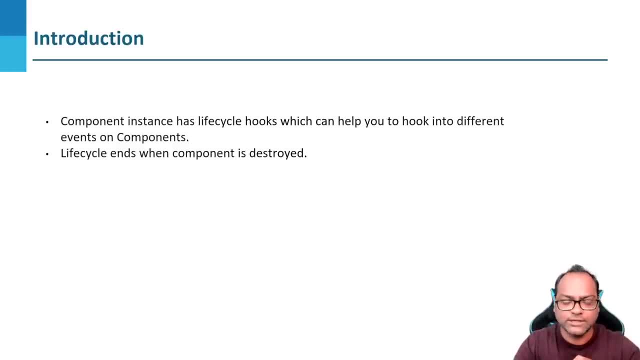 from start, for from creating an instance to destroying an instance. this is how to destroying an instance. this is how to destroying an instance. this is how your entire life cycle looks. looks like your entire life cycle looks. looks like your entire life cycle looks, looks like, and uh, 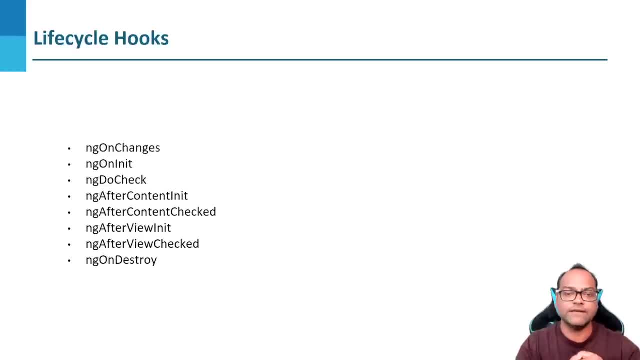 and uh and uh, there are, there are, there are few lifestyle looks. uh sorry, these are few lifestyle looks. uh sorry, these are few lifestyle looks. uh sorry, these are the life cycle looks which are mentioned, the life cycle looks which are mentioned, the life cycle looks which are mentioned here. so you have on changes on in it, do? 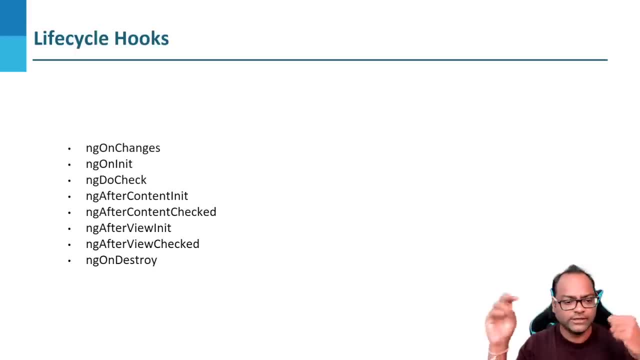 here so you have on changes on in it. do here so you have on changes on in it. do check, check, check. after content in it checked, we need after content in it checked, we need after content in it checked, we need checked and then destroy. so let's uh go. 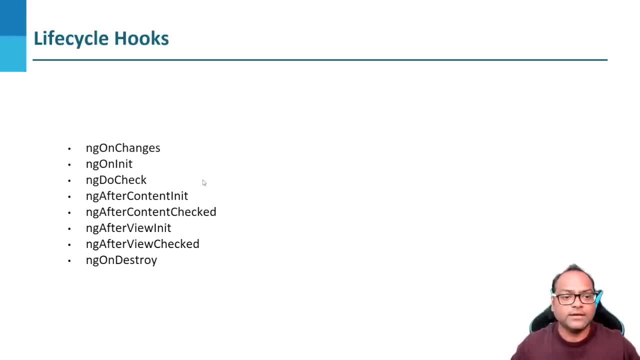 checked and then destroy. so let's uh go checked and then destroy. so let's uh go through each of them one by one, through each of them one by one, through each of them one by one. and yeah, yeah, yeah, and you might have already noticed that, and you might have already noticed that: 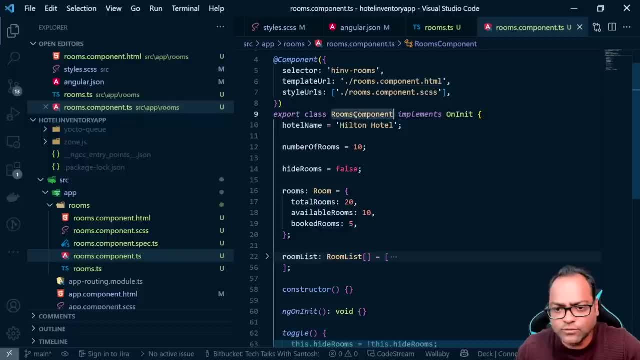 and you might have already noticed that ng on init life cycle hooks already exist. ng on init life cycle hooks already exist. ng on init life cycle hooks already exist on your rooms component. so if you see on your rooms component, so if you see on your rooms component, so if you see this, 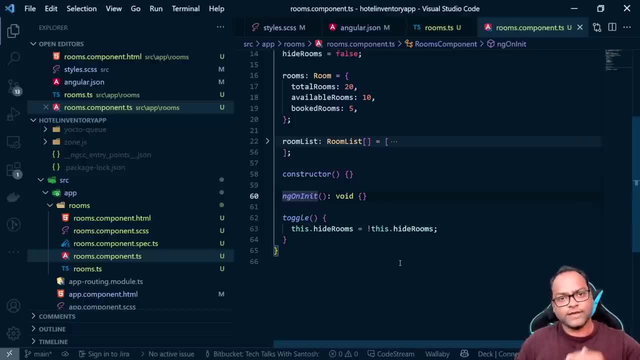 this, this: uh, there is ng on in it. uh, there is ng on in it. uh, there is ng on in it. so in angular for every life cycle looks. so in angular for every life cycle looks. so in angular for every life cycle looks. there is an interface, so, for example, ng: 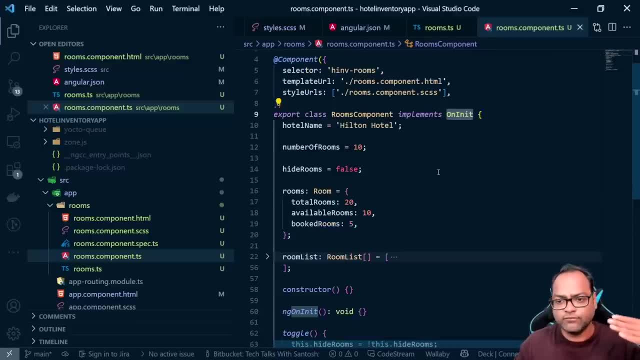 there is an interface, so, for example, ng. there is ng on in it. so, for example, ng on in it has an interface called on init on in it has an interface called on init on in it has an interface called on init. so if i have destroy on ng on destroy, so 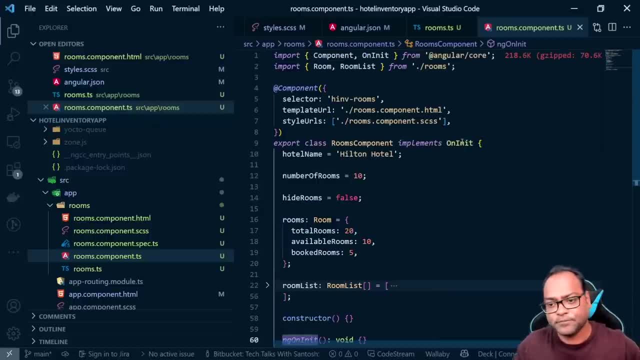 so if i have destroy on ng on destroy so, so if i have destroy on ng on destroy so there is an event called. there is an event called. there is an event called: or an interface called on destroy you can, or an interface called on destroy you can. 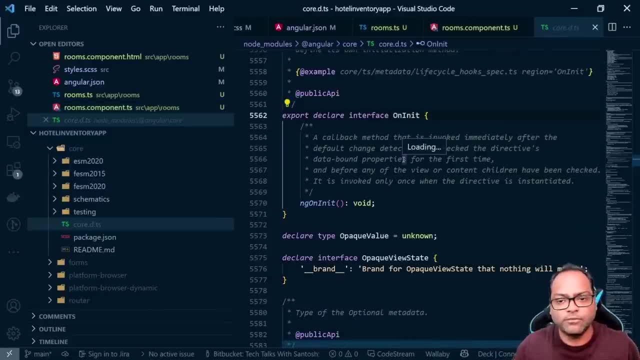 or an interface called on destroy. you can just go to this event and just go to this event. and just go to this event and same f1 or control click and you will go. same f1 or control click and you will go same f1 or control click and you will go inside this to see which event is that. 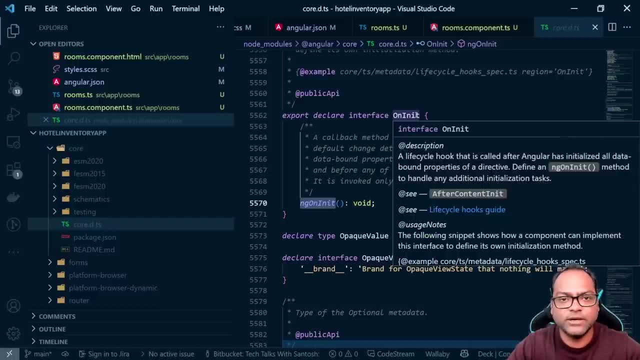 inside this to see which event is that, inside this to see which event is that so. so so ng on in it in earlier days. it was ng on in it in earlier days. it was ng on in it in earlier days. it was optional but optional but optional. but uh, make sure that you implement the. 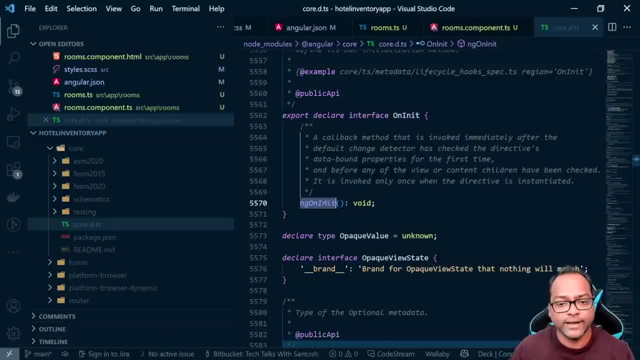 uh, make sure that you implement the? uh, make sure that you implement the interface interface interface whenever you are trying to access, whenever you are trying to access, whenever you are trying to access some of the life cycle looks of your, some of the life cycle looks of your. 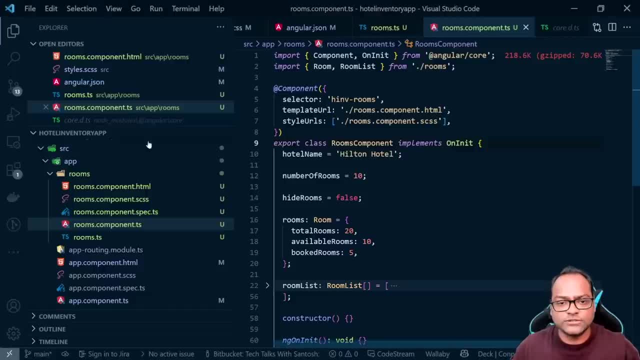 some of the life cycle looks of your component. so component, so component. so let's see what you can achieve using uh. let's see what you can achieve using uh. let's see what you can achieve using uh. ng on it. life cycle- look, but before we ng on it. life cycle- look, but before we. 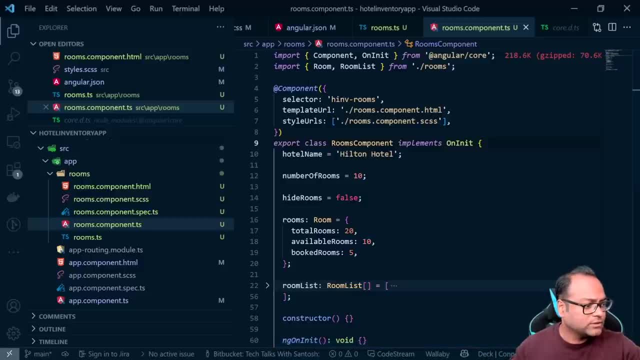 ng on it. life cycle, look, but before we go ahead and do that, before we actually go ahead and do that, before we actually go ahead and do that, before we actually move, move, move. so before, sorry, so before, sorry, so before sorry. before we go ahead and move, uh, do that. 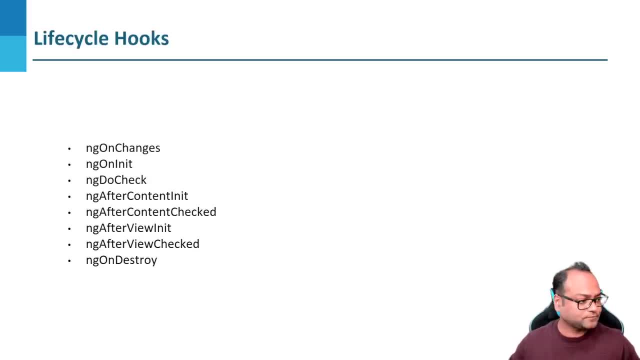 before we go ahead and move. uh, do that. before we go ahead and move, uh, do that before we talk about ng on in it. before we talk about ng on in it, before we talk about ng on in it. here, you will notice that there is also. here, you will notice that there is also. 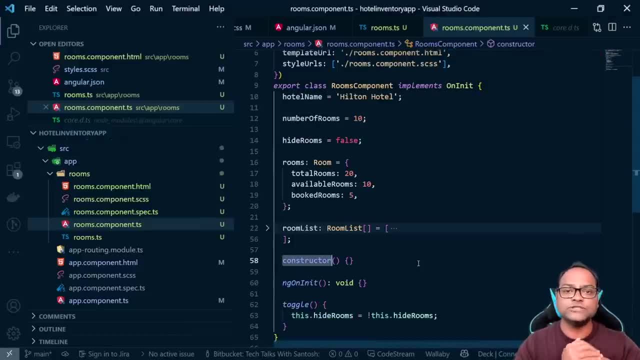 here you will notice that there is also a constructor which is available. so it a constructor which is available. so it a constructor which is available. so it means before even your ng on init event, means before even your ng on init event, means before even your ng on init event gets called. 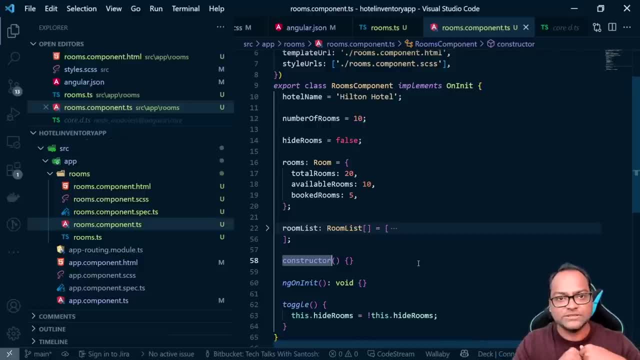 gets called, gets called, your component needs to be initialized. so your component needs to be initialized. so your component needs to be initialized. so this is where it this happens and when this is where it this happens, and when this is where it this happens and when in uh. 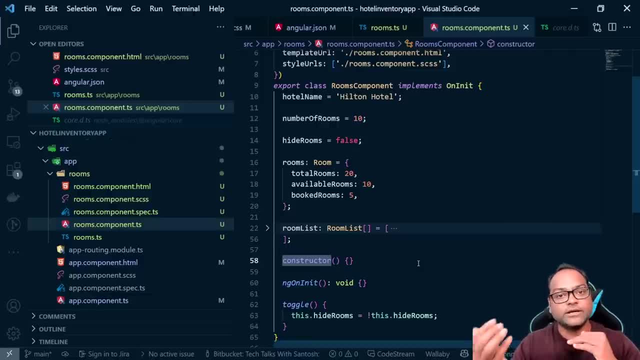 in uh in uh, when it happens actually on your page, uh, when it happens actually on your page, uh, when it happens actually on your page, uh, whenever it gets uh rendered on your, whenever it gets uh rendered on your, whenever it gets uh rendered on your view, at that time constructor will be. 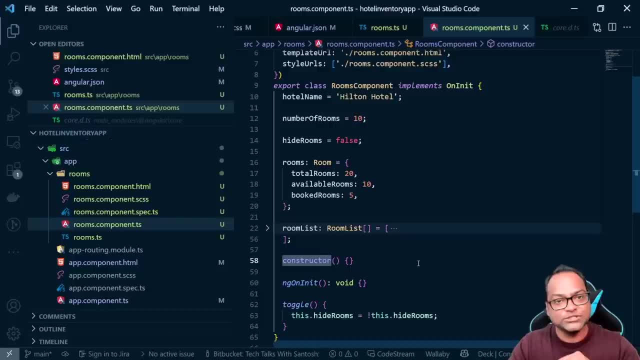 view. at that time, constructor will be view. at that time, constructor will be called and called and called. and just after the constructor is finished, just after the constructor is finished, just after the constructor is finished, your ng on init lifecycle, your ng on init lifecycle, your ng on init lifecycle, ng on init lifecycle, look, will be called. 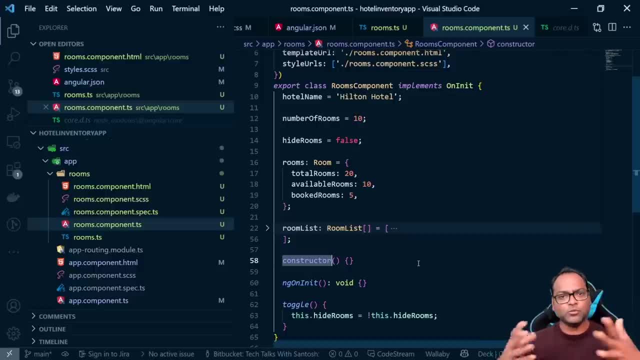 ng on init lifecycle, look will be called ng on init lifecycle, look will be called so. people do uh get confused, okay. if so, people do uh get confused, okay. if so, people do uh get confused, okay. if both are kind of same, that okay once my. both are kind of same, that okay, once my. 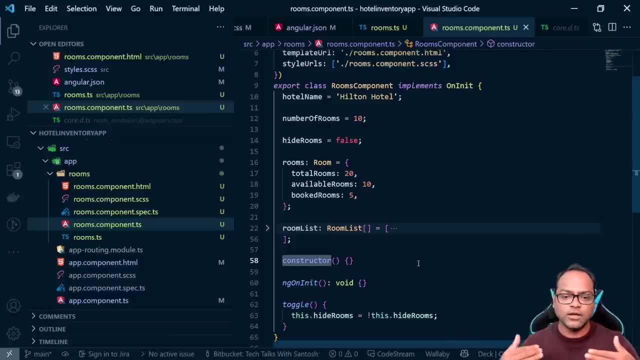 both are kind of same, that, okay, once my component is initialized, i can just look, component is initialized, i can just look component is initialized, i can just look into ng on unit, into ng on unit, into ng on unit, lifecycle, look, lifecycle, look, lifecycle, look. what is the difference between? 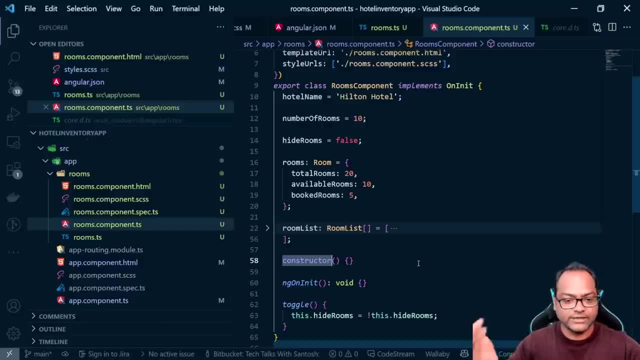 what is the difference between? what is the difference between: constructor- i mean we are. we are saying constructor. i mean we are. we are saying constructor, i mean we are. we are saying that whenever an instance is created, a that whenever an instance is created, a that whenever an instance is created, a constructor is called. 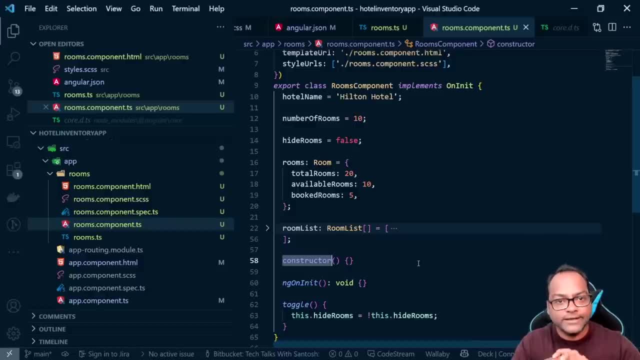 constructor is called. constructor is called: remember ng on. it is where your uh you remember ng on. it is where your uh you remember ng on. it is where your uh you should write, should write, should write. your logic constructor should be used. your logic constructor should be used. 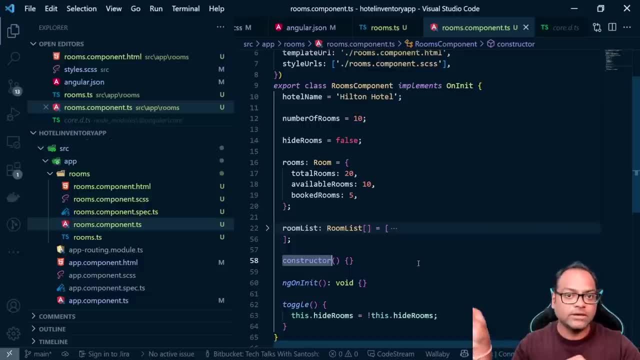 your logic constructor should be used only in case you want to inject some, only in case you want to inject some, only in case you want to inject some services, services, services. this will become. this will be coming. this will become. this will be coming. this will become. this will be coming later on, when we talk about services. 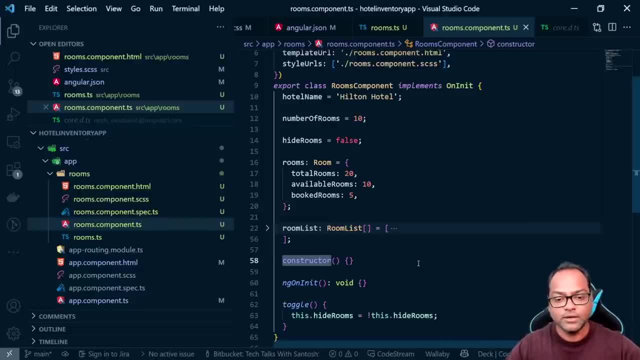 later on when we talk about services, later on when we talk about services. but let's just keep that in my, in, in, in. but let's just keep that in my, in, in, in. but let's just keep that in my, in, in, in your mind, your mind. 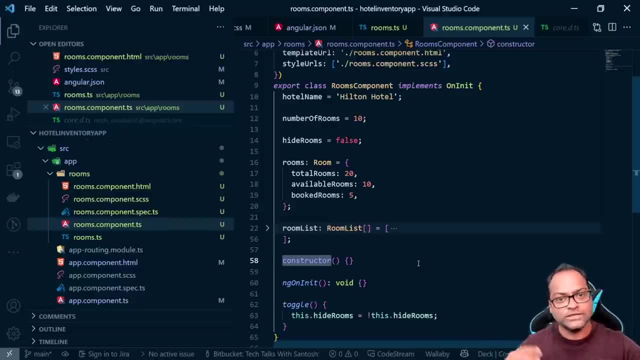 your mind, constructors should not have any constructors should not have any constructors should not have any blocking code. so in case you are writing blocking code, so in case you are writing blocking code, so in case you are writing some blocking code in your constructor, some blocking code in your constructor. 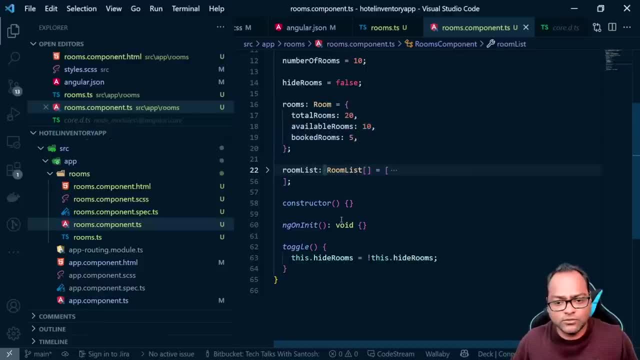 some blocking code in your constructor. just move some property declaration from. just move some property declaration from. just move some property declaration from here to ng on init. so here i'm saying okay this. so here i'm saying okay this. so here i'm saying okay, this room list is equals to. 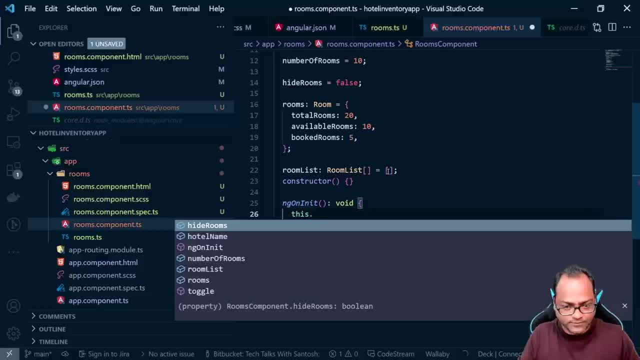 room list is equals to room list is equals to empty array, and then, in ng on it, i will empty array and then, in ng on it, i will empty array and then, in ng on it, i will say this dot, say this dot, say this dot: room list is equals to this records. 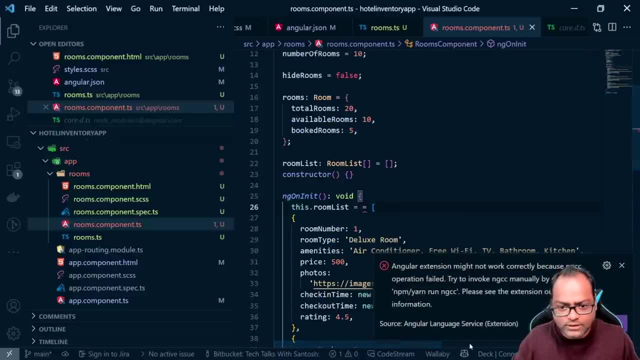 room list is equals to this. records room list is equals to this records, right? so we are just moving, uh, the right, so we are just moving, uh, the right, so we are just moving, uh, the entire array here, entire array here, entire array here, inside engine in it. so, in case you have, 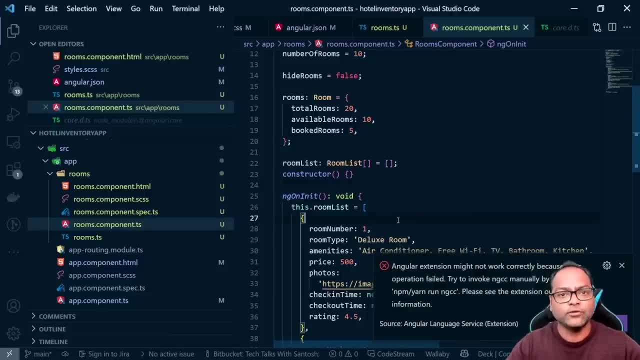 inside engine in it. so in case you have inside engine in it. so in case you have any. let's say you want to load some data any. let's say you want to load some data any. let's say you want to load some data from your api and you want to display. 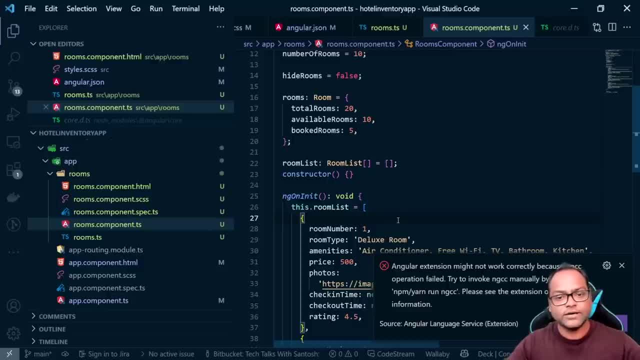 from your api and you want to display from your api and you want to display: uh, that data on your pay view, uh, that data on your pay view, uh, that data on your pay view. you should write that code as part of ng. you should write that code as part of ng. 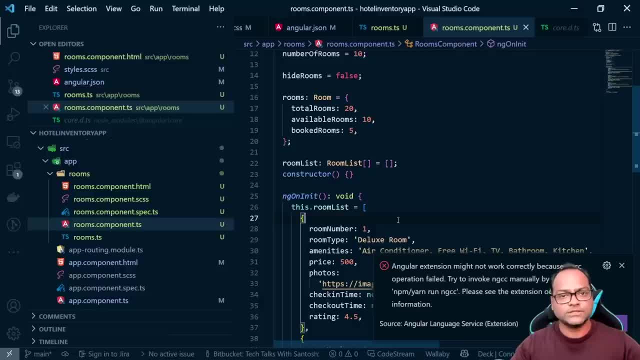 you should write that code as part of ng online life cycle. online life cycle. online life cycle. this should not go into constructor, or this should not go into constructor, or this should not go into constructor or any other life cycle, so ng on it is. any other life cycle, so ng on it is. 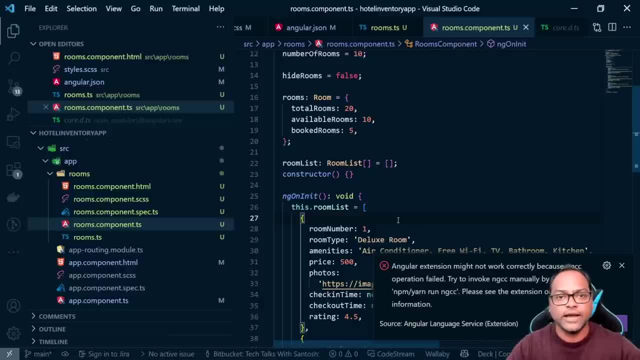 any other life cycle, so ng on. it is something where we are saying that okay, something where we are saying that okay, something where we are saying that okay, now my component is initialized, now my component is initialized, now my component is initialized and just after my component is. 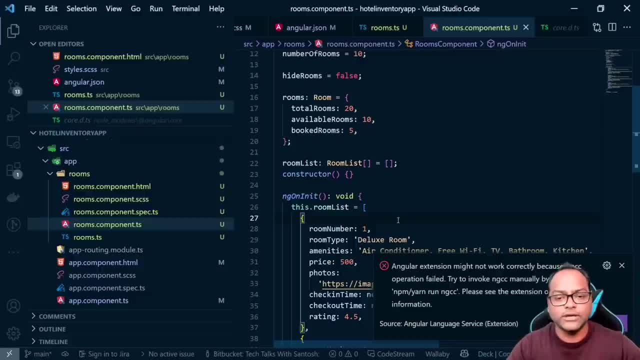 and just after my component is and just after my component is initialized, you want to do anything initialized. you want to do anything initialized. you want to do anything. just add that code into ng on any. just add that code into ng on any. just add that code into ng on any lifestyle. look, so let's go ahead and 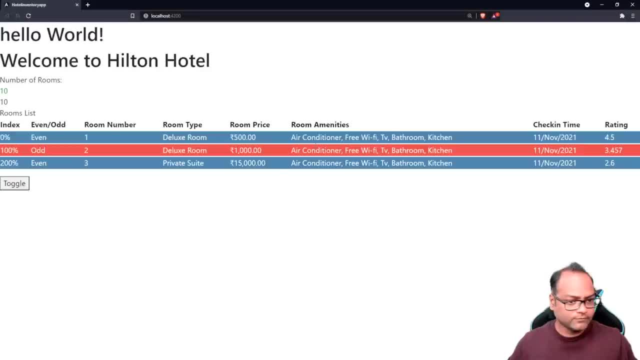 lifestyle look, so let's go ahead. and lifestyle look, so let's go ahead and verify our, verify our, verify our view. and here we are. i mean there is no, and here we are. i mean there is no, and here we are. i mean there is no changes. 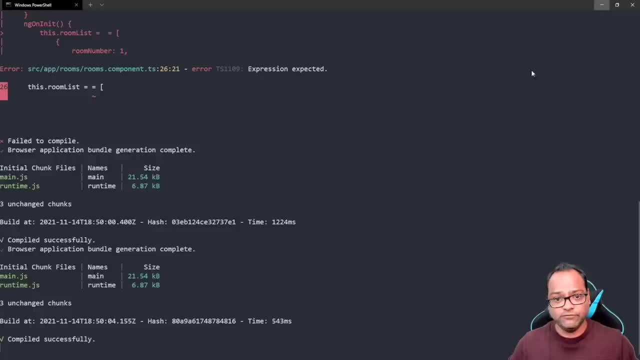 changes, changes and our code is compiled as well. so this and our code is compiled as well. so this and our code is compiled as well. so this is all about engineering. we will be. is all about engineering. we will be. is all about engineering we will be usually utilizing. 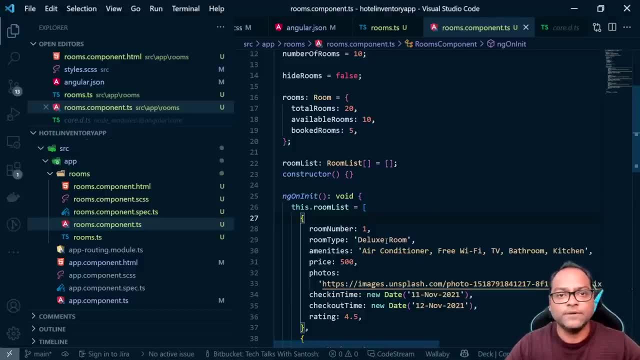 usually utilizing- usually utilizing, we will be utilizing ng on it life cycle. we will be utilizing ng on it life cycle. we will be utilizing ng on it life cycle looks in future whenever we looks in future, whenever we looks in future, whenever we start implementing our services and start. 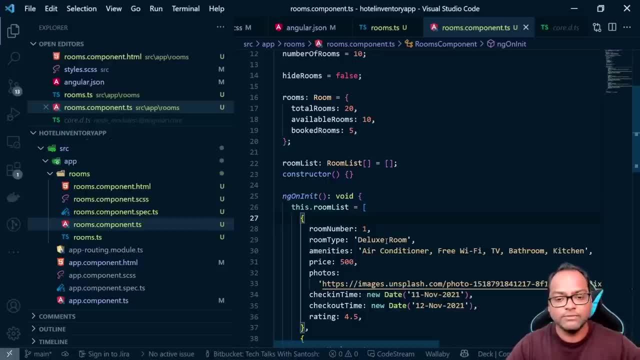 start implementing our services and start start implementing our services and start getting the data from the api. so we'll getting the data from the api, so we'll getting the data from the api. so we'll see some use cases where we will be, see some use cases where we will be. 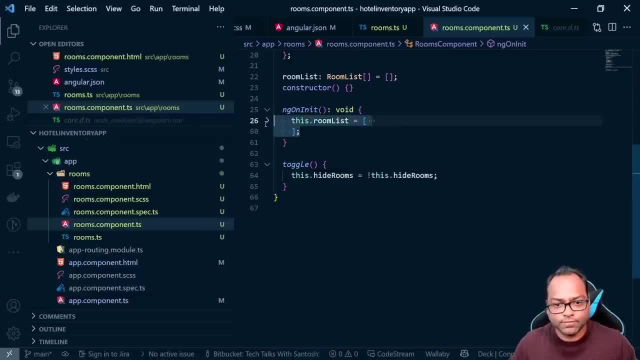 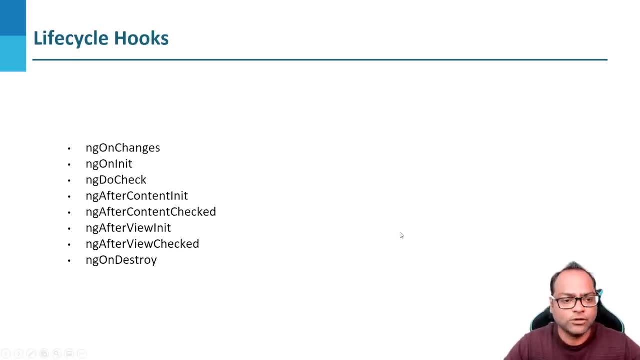 see some use cases where we will be using it now. let's go back and talk about other. now let's go back and talk about other. now let's go back and talk about other. life cycle looks so you might be wondering. i mean i said so you might be wondering. i mean i said 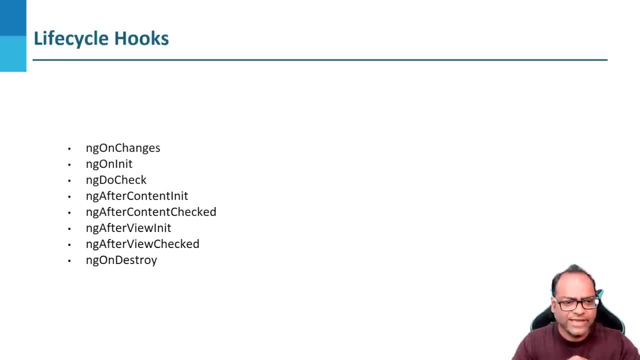 so you might be wondering. i mean, i said ng on unit is the first life cycle event. ng on unit is the first life cycle event. ng on unit is the first life cycle event, then why i have mentioned it second year? then why i have mentioned it second year? 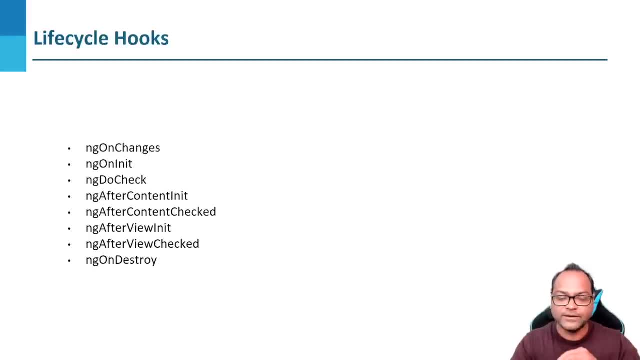 then why i have mentioned it second year? of course, that's, of course, that's, of course, that's. that should be the question in your mind, that should be the question in your mind. that should be the question in your mind right now, right now, right now. so we have ng on changes, which is before. so we have ng on changes which is before, so we have ng on changes which is before. ng on unit. remember in this life cycle. ng on unit. remember in this life cycle. ng on unit. remember in this life cycle: looks. constructor is the first one which looks. constructor is the first one which. 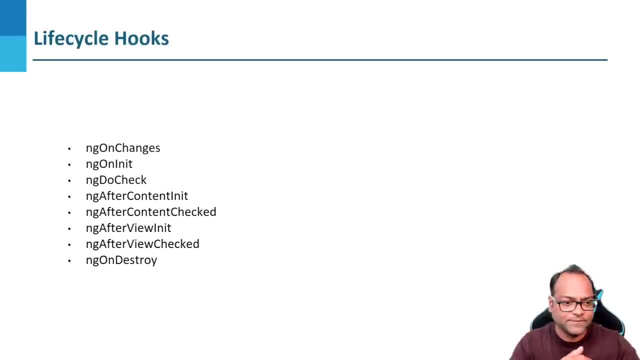 looks, constructor is the first one which will be called every will be called every will be called every for every component, once they are for every component, once they are for every component, once they are initialized, initialized, initialized. so we have ng on changes before ng on in. so we have ng on changes before ng on in. 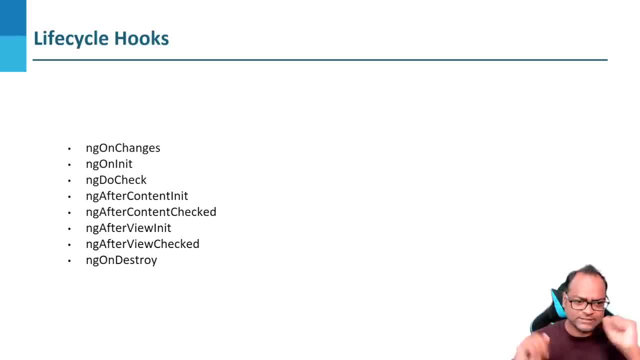 so we have ng on changes before ng on in it. then we have ng to check it. then we have ng to check it, then we have ng to check. let's uh go ahead and talk about uh. let's uh go ahead and talk about uh. let's uh go ahead and talk about uh. so 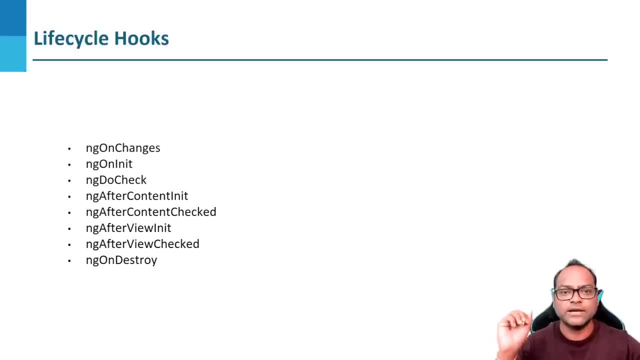 so so there are two topics which will go, there are two topics which will go. there are two topics which will go: parallely here, so life cycle looks, and parallely here, so life cycle looks, and parallely here, so life cycle looks, and there will be something known as component. 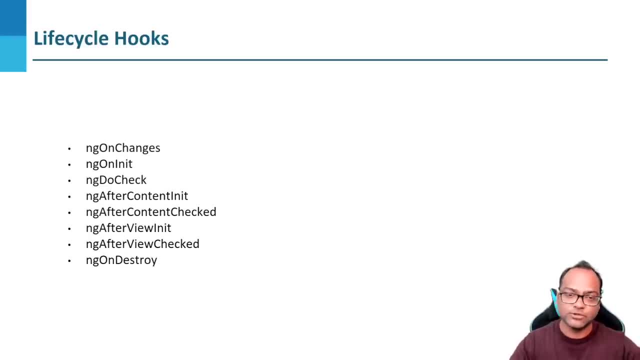 there will be something known as component. there will be something known as component: communication, communication, communication, this, this, two topics. i generally take it this, this two topics, i generally take it this, this two topics, i generally take it parallely because they parallely, because they parallely, because they, they need each other. i mean they, uh, they. 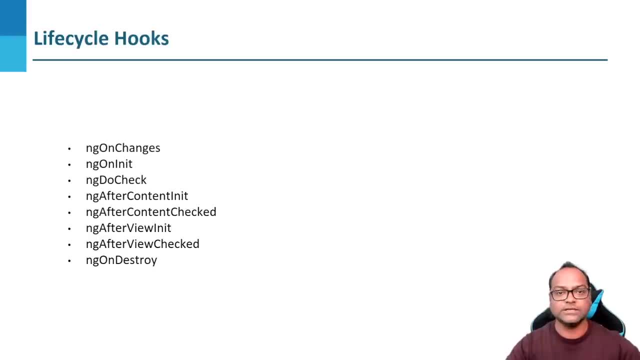 they need each other. i mean they, uh, they. they need each other. i mean they, uh. they needs to be understand. uh needs to be understand, uh needs to be understand. uh, while talking about life cycle looks, and while talking about life cycle looks, and while talking about life cycle looks, and then you, 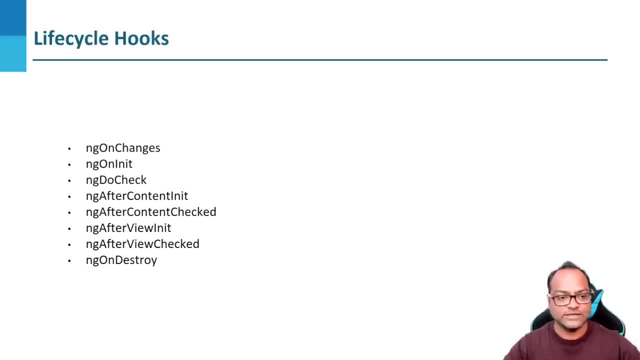 then you, then you needs to know about component life cycle, needs to know about component life cycle, needs to know about component life cycle. sorry component interaction as well. sorry component interaction as well. sorry component interaction as well. so this ng on changes actually uh is. so this ng on changes: actually uh is. 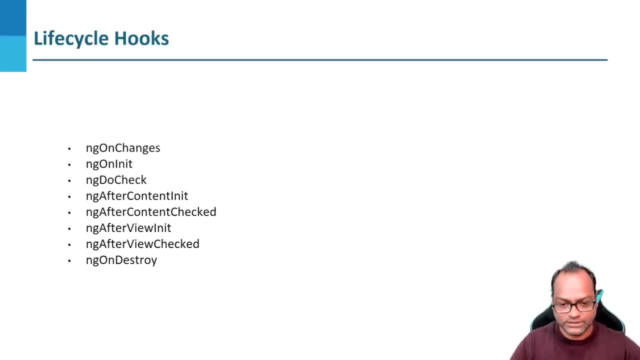 so this ng on changes actually, uh is related to one of the, related to one of the, related to one of the ways you can do component ways you can do component ways you can do component communication, communication, communication. let me just go back and talk a little. let me just go back and talk a little. 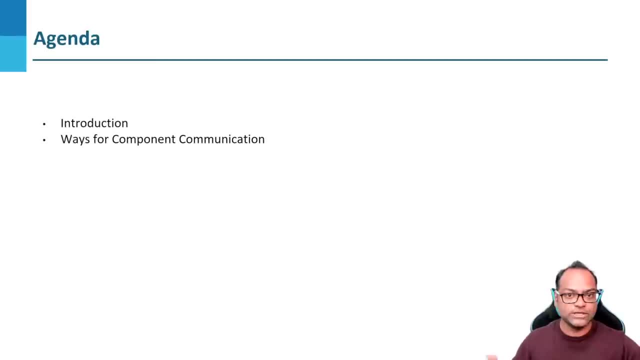 let me just go back and talk a little bit about component communication. bit about component communication, bit about component communication. because we will be using uh component, because we will be using uh component, because we will be using uh component communication, communication, communication in our code right now. so what we will 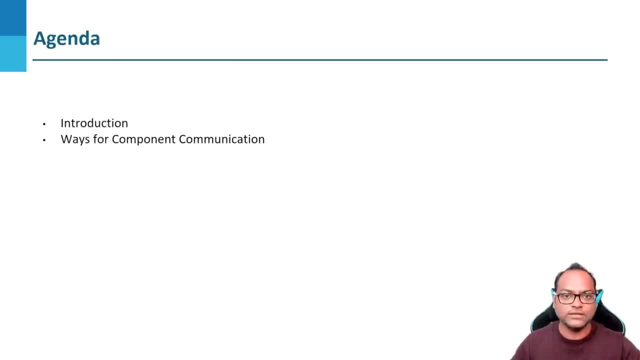 in our code right now. so what we will in our code right now, so what we will be talking about here is be talking about here is be talking about here- is just theory. i mean we are going to see just theory. i mean we are going to see. 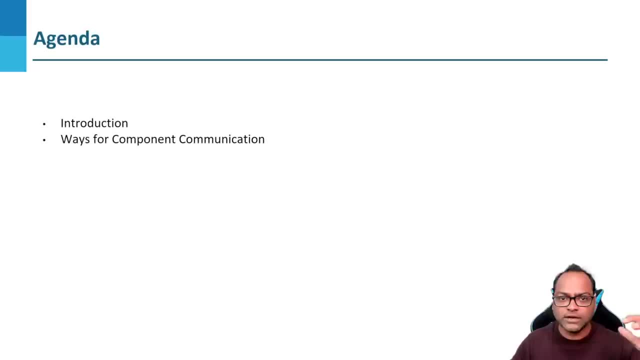 just theory. i mean, we are going to see the examples, so let's introduce, and then the examples, so let's introduce, and then the examples, so let's introduce, and then there are ways for component, there are ways for component, there are ways for component, communication, communication, communication. we will be doing this parallel right. 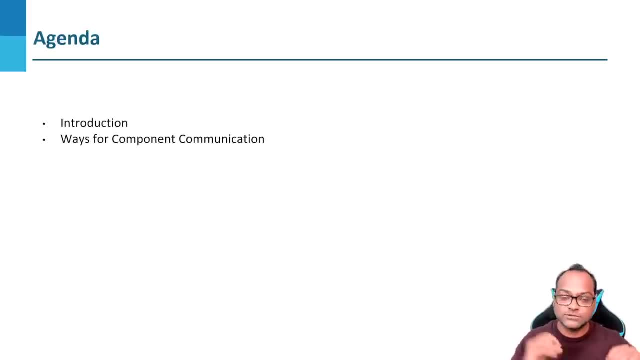 we will be doing this parallel right. we will be doing this parallel right. so ways for component communication, so ways for component communication. so ways for component communication. we will relate to the component life, we will relate to the component life, we will relate to the component life cycle. look so in case. 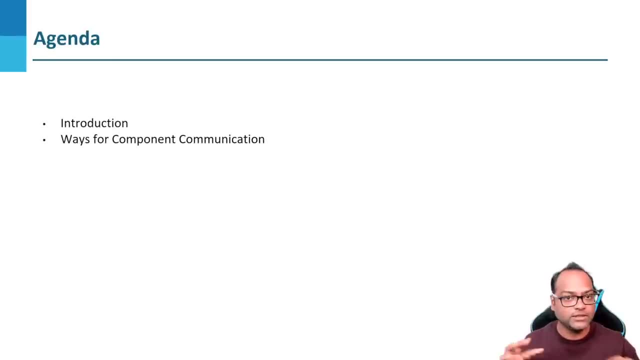 cycle. look so in case. cycle. look so in case you write your real-time code. you know you write your real-time code. you know you write your real-time code. you know what needs to be done, rather than just what needs to be done, rather than just what needs to be done, rather than just doing something blindly so. 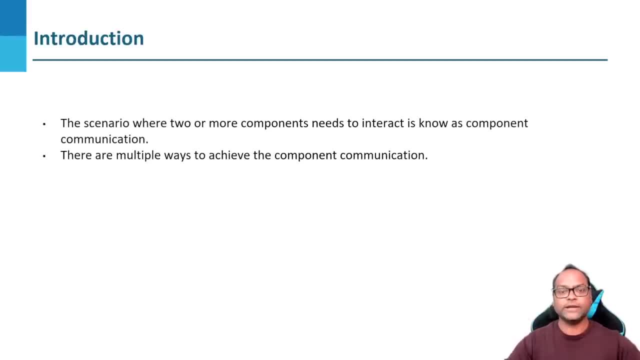 doing something blindly so doing something blindly. so there we are. right now we have two there. we are right now, we have two there we are right now we have two components: app component and components. app component and components. app component and your rooms component. what in case they? your rooms component. what in case they your rooms component. what in case they want to actually interact with each other, want to actually interact with each other, want to actually interact with each other? how we can do that, that's what. how we can do that, that's what. 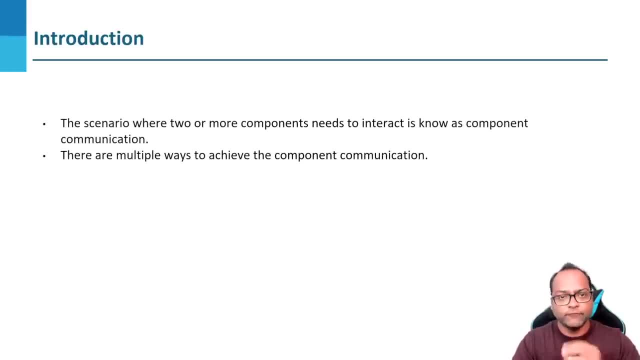 how we can do that. that's what communication- uh component communication, uh, component communication, uh component communication- is all about. communication is all about communication is all about- we also said that uh in future- what we also said that uh in future, what we also said that uh in future, what we will be. 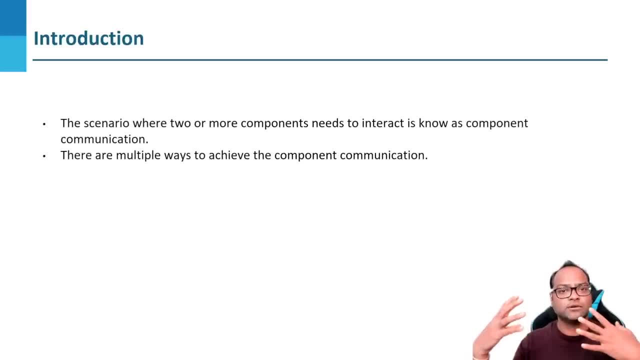 we will be. we will be. we also said in future what we will be. we also said in future what we will be. we also said in future what we will be doing is we will be creating a lot of doing is we will be creating a lot of. 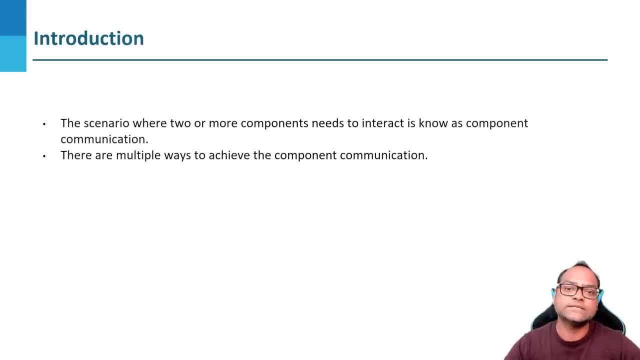 doing is we will be creating a lot of html reusable html tag. that's what html reusable html tag. that's what html reusable html tag. that's what component is. component is. component is what in case i want to create those. what, in case i want to create those? 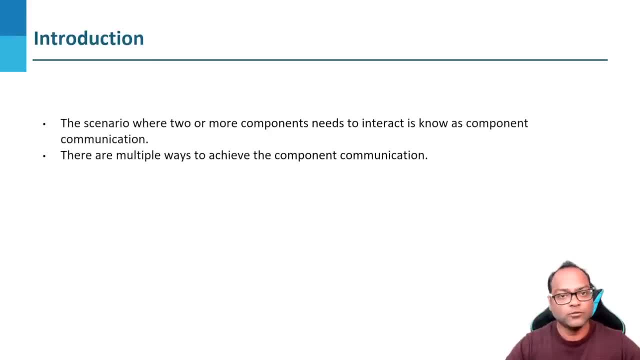 what in case? i want to create those reusable tags, and then i can use it reusable tags, and then i can use it reusable tags, and then i can use it anywhere, anywhere, anywhere. who will be passing the data, of course. who will be passing the data, of course? 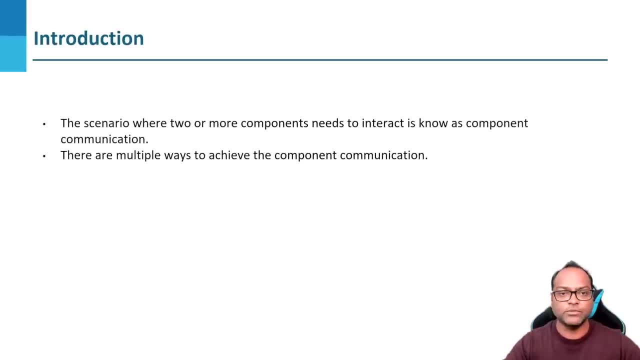 who will be passing the data? of course, someone has to interact with that. someone has to interact with that. someone has to interact with that particular component. right, that's a particular component. right, that's a particular component. right, that's a reusable component, so it cannot contain. reusable component, so it cannot contain. 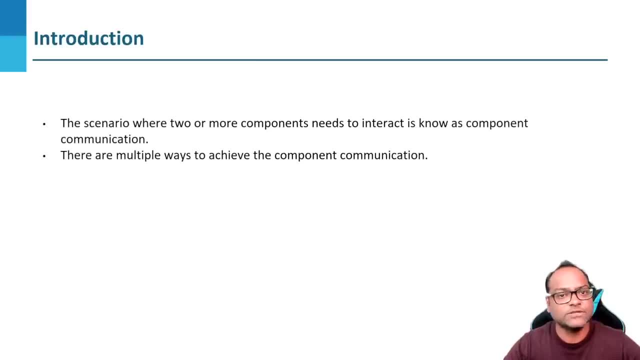 reusable component, so it cannot contain its own information. it has to rely on its own information. it has to rely on its own information. it has to rely on some information which is coming from, some information which is coming from, some information which is coming from somewhere else- that's your another. 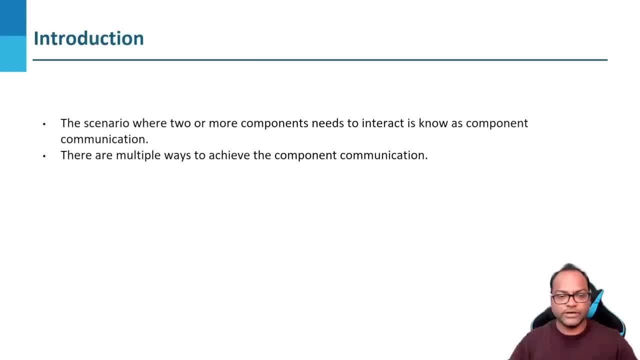 somewhere else that's your another, somewhere else that's your another component, component, component. this is component communication. this is component communication. this is component communication. so multiple components interacting with, so multiple components interacting with, so multiple components interacting with each other, but there are multiple ways each other, but there are multiple ways. 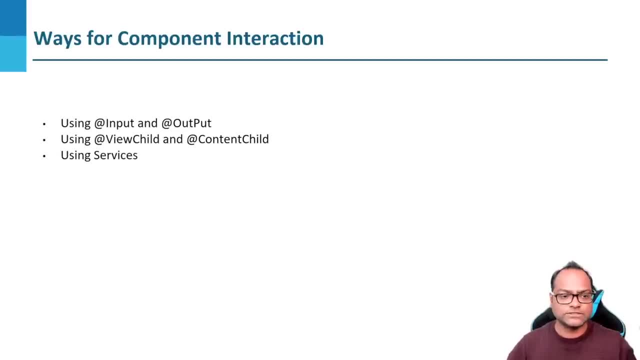 each other. but there are multiple ways now, now, now. so there are three ways which we so. there are three ways which we so there are three ways which we generally use. so first is using input generally use. so first is using input generally use. so first is using input and output. second is using view children. 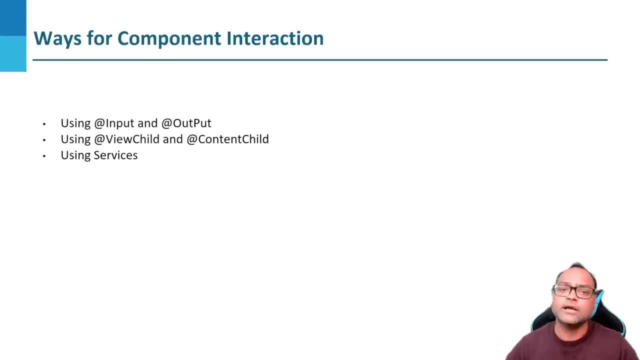 and output. second is using view children and output. second is using view children or content children: sorry view child or or content children- sorry view child or or content children. sorry view child or content child. and third one is using content child and third one is using content child and third one is using service. 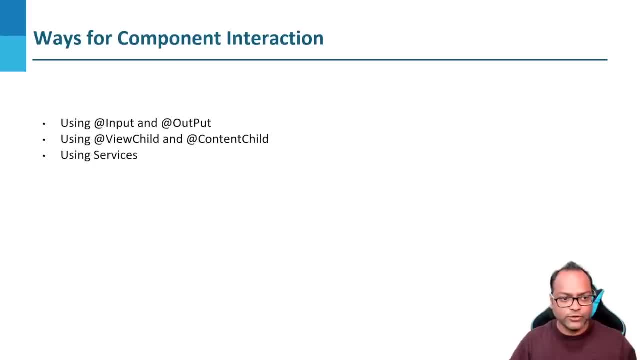 service service. now, as we talk about ng on changes, we now as we talk about ng on changes, we now, as we talk about ng on changes, we are going to use the component, are going to use the component, are going to use the component communication using input and output. 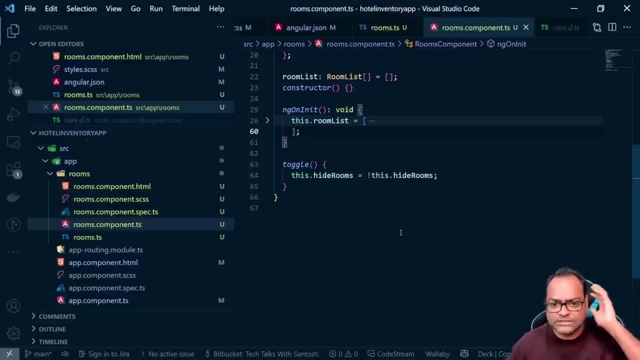 communication using input and output. communication using input and output. so let's try to create a scenario first. so let's try to create a scenario first. so let's try to create a scenario first. so, in this uh application right now, if so, in this uh application right now, if 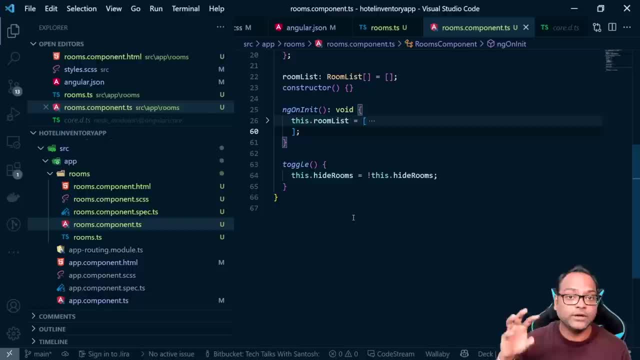 so in this uh application right now, if you see, you see, you see now we uh, you are also going to learn now we uh. you are also going to learn now we uh. you are also going to learn how you can actually split your, how you can actually split your. 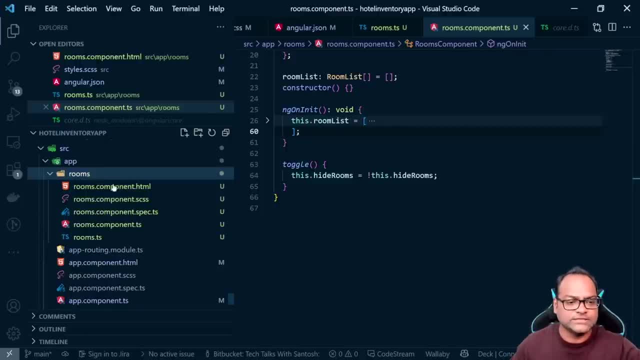 how you can actually split your big components into smaller components, big components into smaller components, big components into smaller components. so if you see this html, so if you see this html, so if you see this html which has like like 43 lines of code, which has like like 43 lines of code, 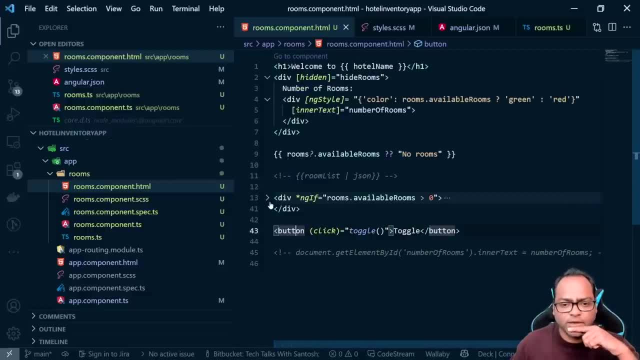 which has like like 43 lines of code right now, 43 lines of html, right now 43 lines of html, right now 43 lines of html. if you see, uh, if you think about this, if you see, uh, if you think about this, if you see, uh, if you think about this table. 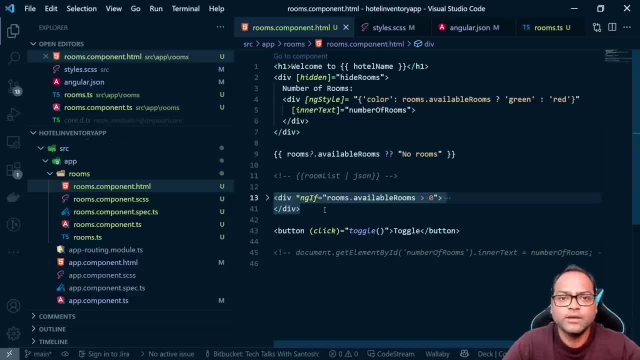 table table. i think this table can be another. i think this table can be another. i think this table can be another component, component, component. the reason being i can just remove this, the reason being i can just remove this, the reason being i can just remove this logic and keep my component smaller. 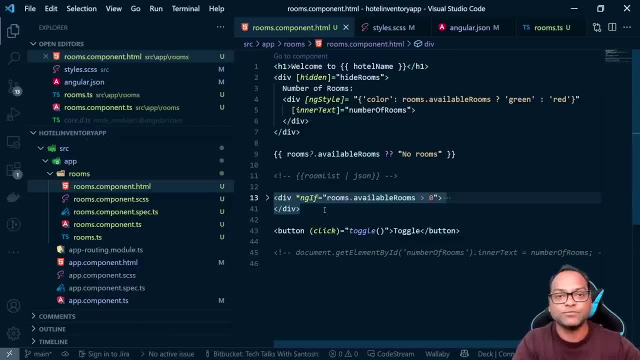 logic and keep my component smaller. logic and keep my component smaller. that's what we uh often do, right, whenever. that's what we uh often do, right, whenever. that's what we uh often do, right, whenever we talk about single responsibility. we talk about single responsibility. we talk about single responsibility, and this has nothing to do with rooms. and this has nothing to do with rooms. and this has nothing to do with rooms. right, i can actually go ahead and display. right, i can actually go ahead and display. right, i can actually go ahead and display a lot of information, and then i can just a lot of information, and then i can just 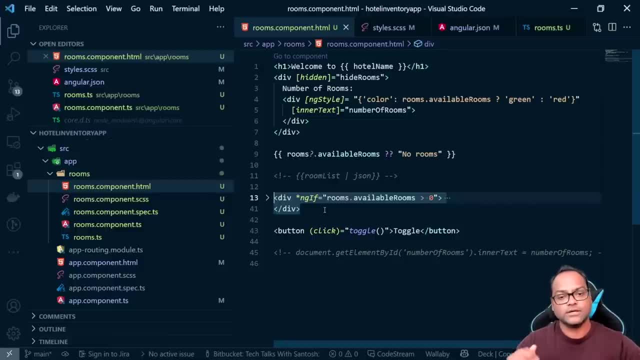 a lot of information and then i can just keep this logic separate. keep this logic separate. keep this logic separate. testing a good idea? the answer is no. testing a good idea? the answer is no. testing a good idea? the answer is no. what we can do, we can actually create a. 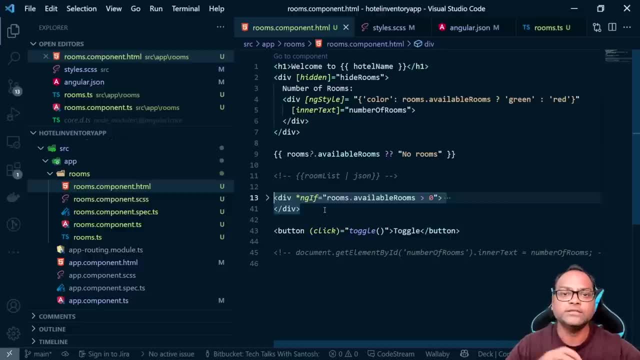 what we can do. we can actually create a. what we can do, we can actually create a reusable sql tag. put this reusable sql tag, put this reusable sql tag, put this somewhere else and just pass the data somewhere else. and just pass the data somewhere else and just pass the data. that's it. that's what we are going to do. 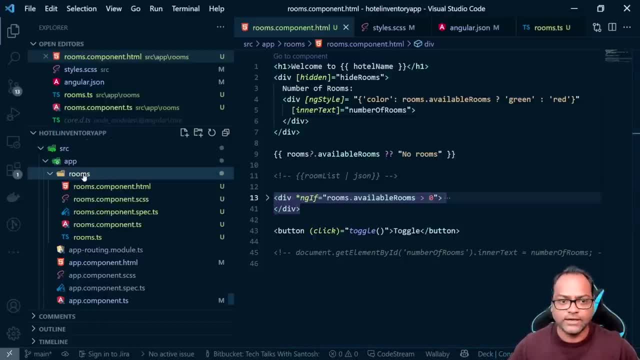 that's it. that's what we are going to do. that's it. that's what we are going to do now, now, now. so let's go ahead and create a component. so let's go ahead and create a component. so let's go ahead and create a component, and 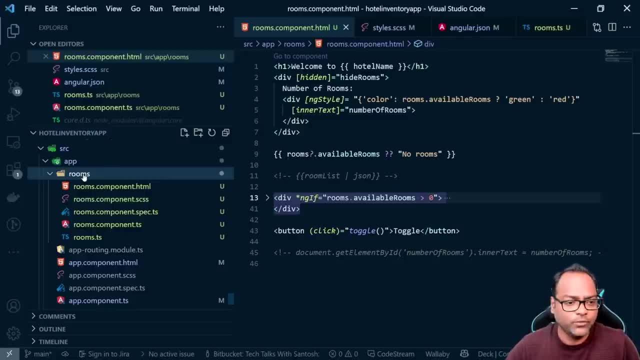 and and. as this component is related to rooms, as this component is related to rooms. as this component is related to rooms, i'll put this inside rooms. i'll call it. i'll put this inside rooms. i'll call it. i'll put this inside rooms. i'll call it. call it as rooms list. 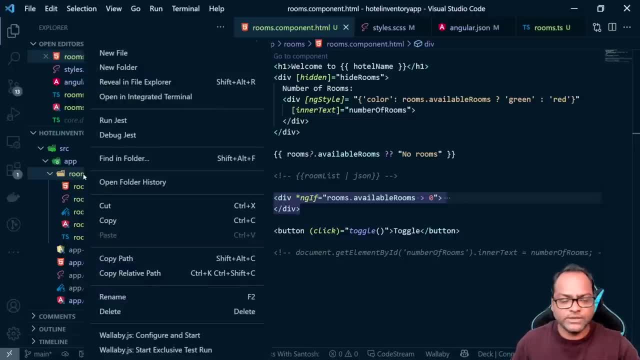 call it as rooms list. call it as rooms list. so here in case you want to create this. so here in case you want to create this. so here in case you want to create this component inside this particular folder, component inside this particular folder, component inside this particular folder. i can just go ahead and say: 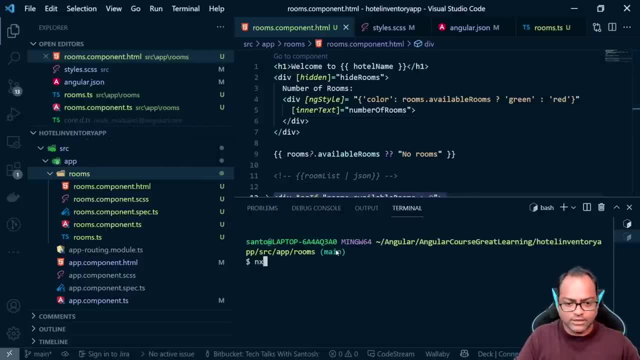 i can just go ahead and say: i can just go ahead and say: open an integrated terminal, and open an integrated terminal, and open an integrated terminal and to create a new component. we already to create a new component, we already to create a new component, we already learned the command. so i can say: ng. 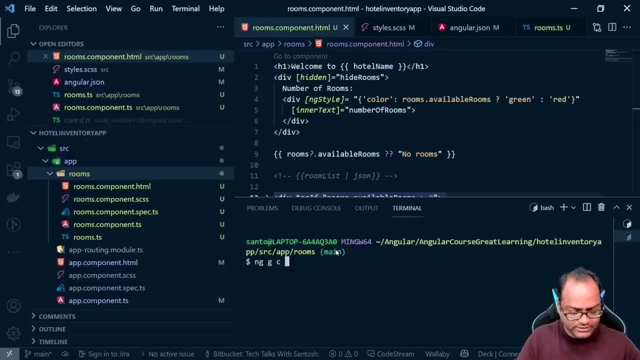 learned the command so i can say ng. learned the command so i can say ng g c, which is ng generate component, g c, which is ng generate component, g c, which is ng generate component. and then i can say rooms hyphen list and then i can say rooms, hyphen list. 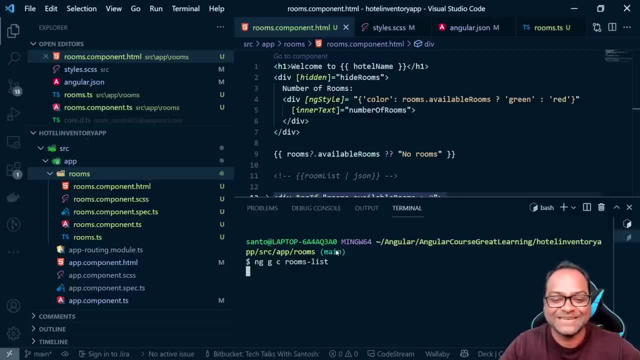 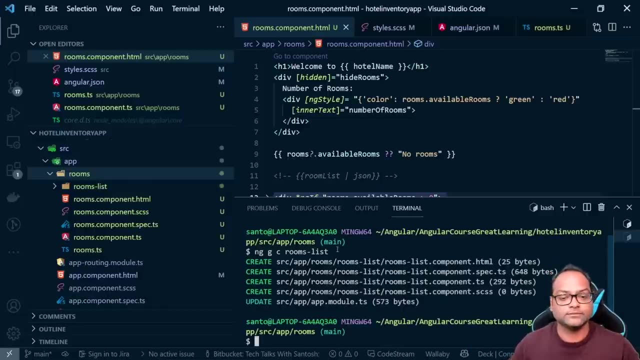 and then i can say: rooms hyphen list. i'm not sure why i keep. i'm not sure why i keep, i'm not sure why i keep making the mistake of making the mistake of making the mistake of rooms then. so now we have this rooms list. 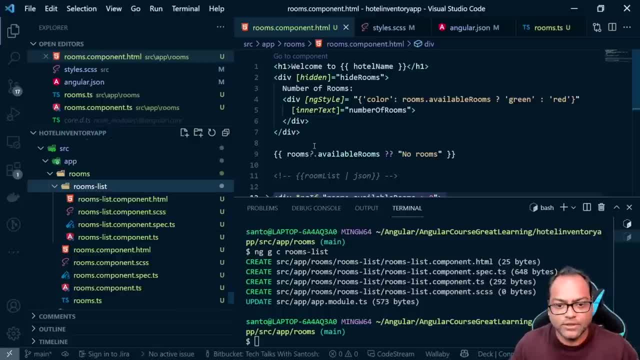 then. so now we have this rooms list then. so now we have this rooms list, folder and folder and folder and all four files as we discussed earlier, all four files as we discussed earlier, all four files as we discussed earlier. now, let's do, uh, one thing, so we will. 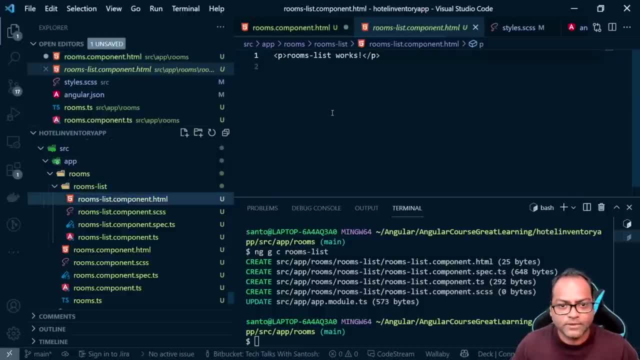 now, let's do uh one thing, so we will. now, let's do uh one thing, so we will remove this, remove this, remove this logic from here, logic from here, logic from here, and put it here, and put it here, and put it here, so my entire table, uh logic, i mean to. 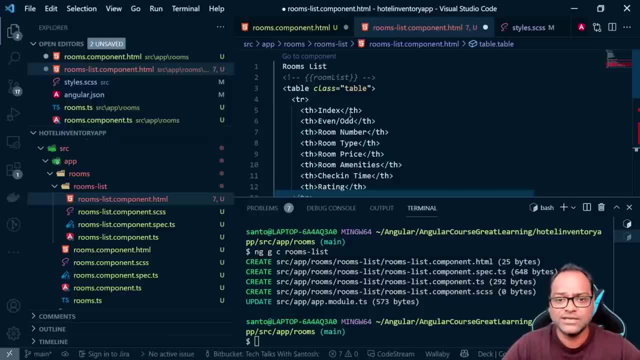 so my entire table. uh logic, i mean to so my entire table. uh logic, i mean to render the table or render the rooms. render the table, or render the rooms. render the table or render the rooms. list is not part of it. i mean it's not. list is not part of it, i mean it's not. 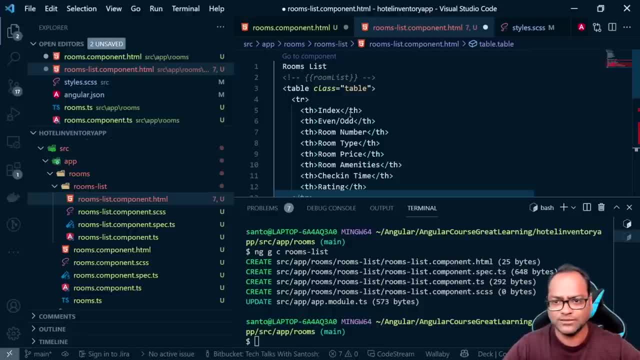 list is not part of it. i mean it's not part of rooms component. it's part of part of rooms component. it's part of part of rooms component. it's part of my rooms list component makes sense, right. my rooms list component makes sense, right. my rooms list component makes sense, right, i mean it. 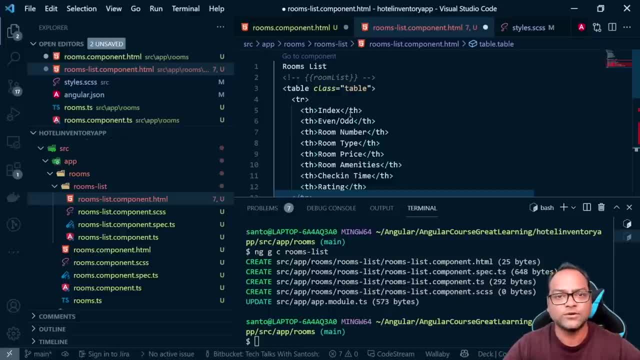 i mean it. i mean it. it even tells you what it is supposed to. it even tells you what it is supposed to. it even tells you what it is supposed to do. it is supposed to list the rooms. do it is supposed to list the rooms? do it is supposed to list the rooms? now let's talk about the data. so we have 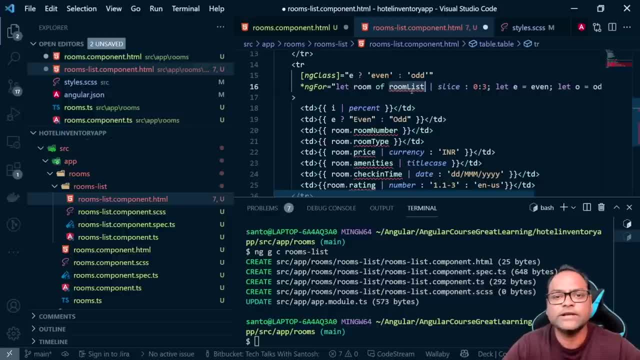 now let's talk about the data. so we have. now let's talk about the data. so we have, okay, rooms list, okay rooms list, okay, rooms list, and uh, we don't have the data right now. and uh, we don't have the data right now. and uh, we don't have the data right now. so we 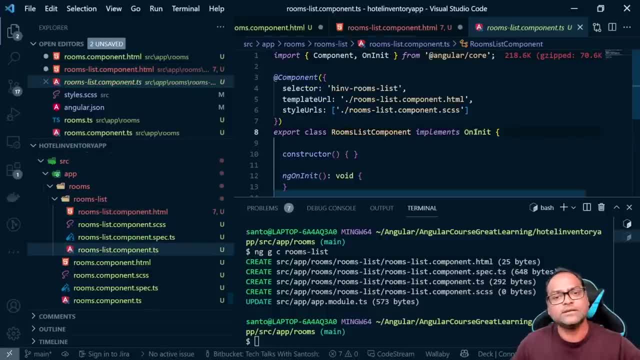 so we so we want to pass the data. so let's see how want to pass the data. so let's see how want to pass the data. so let's see how we can do that. we can do that. we can do that. as we said, we will be using input and 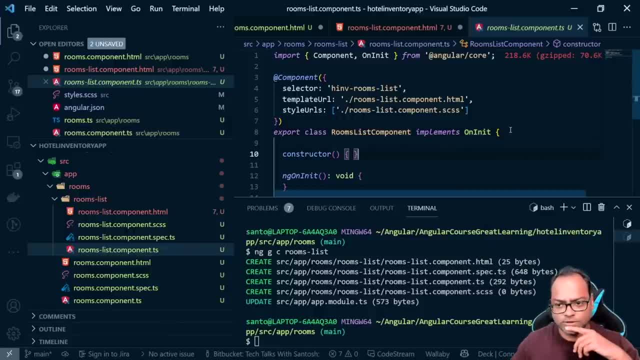 as we said, we will be using input and, as we said, we will be using input and output, output, output. so now let's try to understand both. here we want to get the data. here we want to get the data. here we want to get the data, which means i want to get the input. so 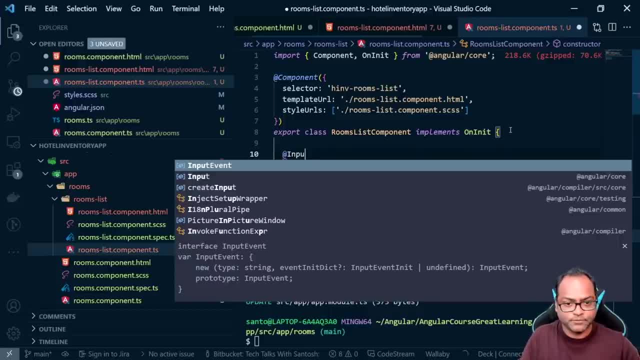 which means i want to get the input. so, which means i want to get the input. so what we will be, what we will be, what we will be doing is we will be creating an input. doing is we will be creating an input. doing is we will be creating an input using accurate input, which is a. 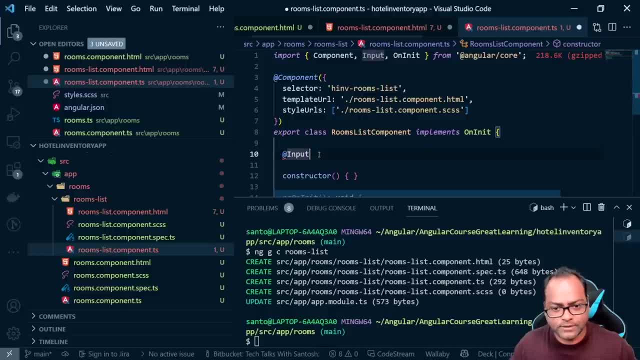 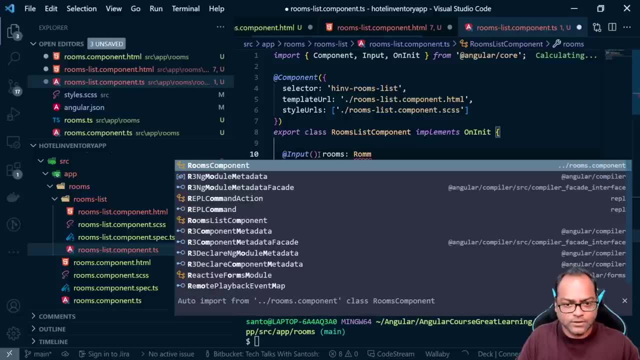 using accurate input, which is a using accurate input. which is a decorator, decorator, decorator, sorry, which is a decorator and i can sorry which is a decorator and i can sorry which is a decorator and i can call it as, call it as, call it as rooms, which is type of. 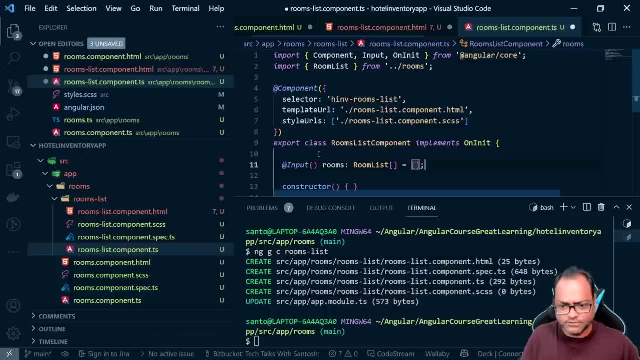 rooms list array is equals to. i mean i rooms list array is equals to. i mean i rooms list array is equals to: i mean i have an empty array by default, have an empty array by default, have an empty array by default. so we are saying: make this rooms. 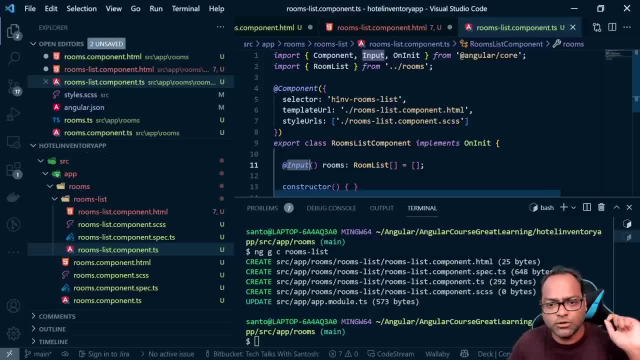 so we are saying: make this rooms. so we are saying: make this rooms. property as an valid html property on property, as an valid html property on property, as an valid html property on this html element. this is what we are, this html element, this is what we are. 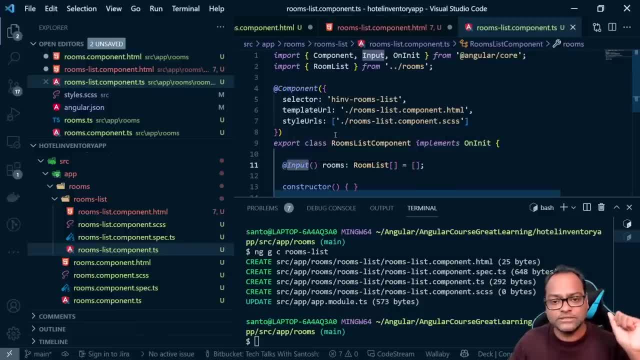 this html element. this is what we are doing here, doing here, doing here: remember whenever you add input tag, it remember, whenever you add input tag, it remember. whenever you add input tag, it means this property rooms becomes, and means this property rooms becomes, and means this property rooms becomes and becomes an property on top of this html. 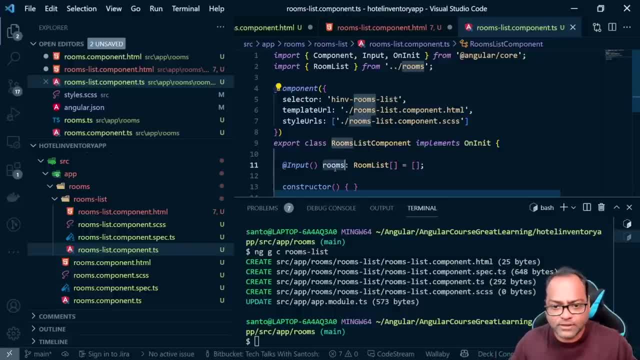 becomes an property on top of this html, becomes an property on top of this html: tag, tag, tag. so we can pass the data now. so we can pass the data now. so we can pass the data now. few need a few. things needs to be. few need a few. things needs to be. 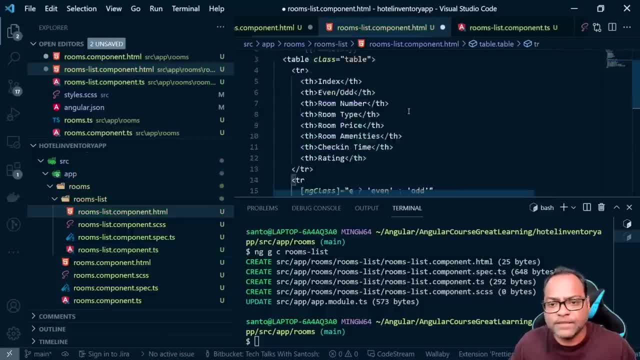 few need a few, things needs to be changed. so, rather than rooms list, i will changed. so, rather than rooms list, i will changed. so, rather than rooms list, i will be saying rooms, be saying rooms, be saying rooms, and that's it. so now all the errors are. 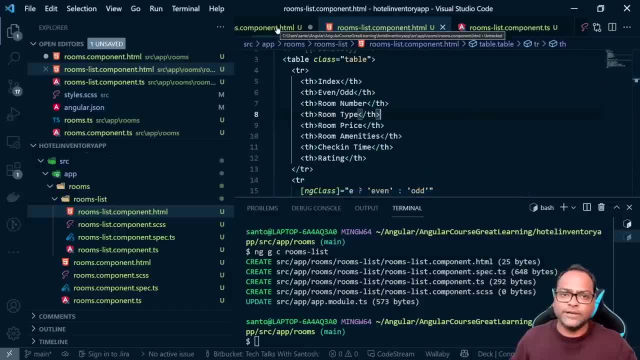 and that's it. so now all the errors are, and that's it. so now all the errors are gone, gone, gone now. let's try to use this component in now. let's try to use this component in now. let's try to use this component in my parent component. 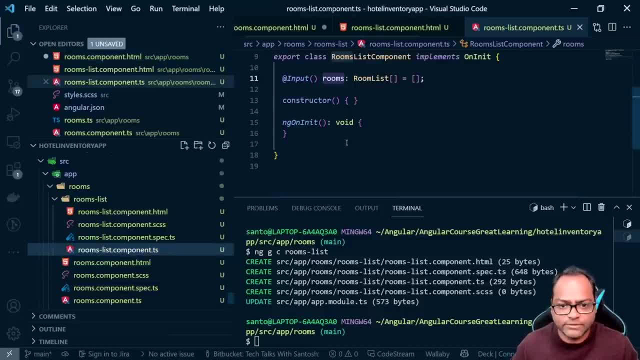 my parent component. my parent component. this is where we want to display that. this is where we want to display that. this is where we want to display that component. so we know the html tag component. so we know the html tag component. so we know the html tag. yes, we do so. i'll copy this. 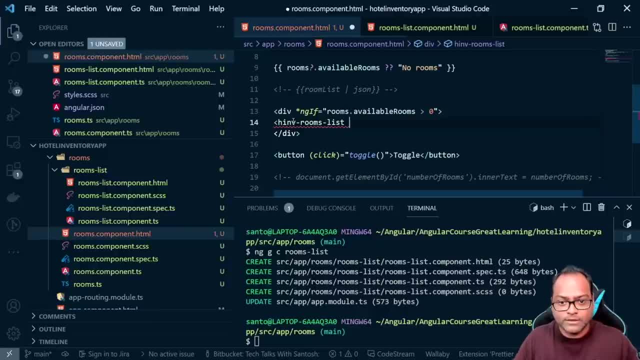 yes, we do so, i'll copy this. yes, we do so. i'll copy this html tag here and, as i said, the rooms is the valid and, as i said, the rooms is the valid and, as i said, the rooms is the valid property which is added here. so i'll say: property which is added here. so i'll say property which is added here. so i'll say rooms. you can see uh due to angular rooms. you can see uh due to angular rooms. you can see uh due to angular language service. we are getting in language service. we are getting in. 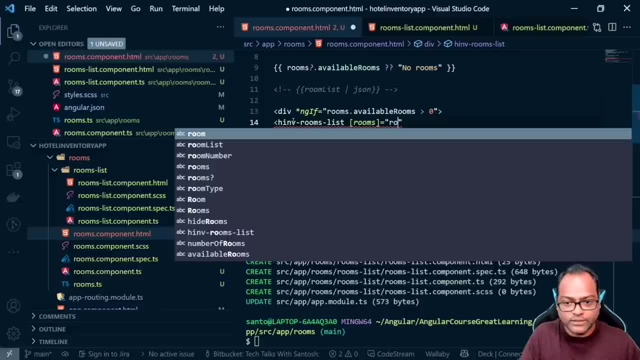 language service we are getting in. intellisense is equals to now we know intellisense is equals to now we know intellisense is equals to now we know that the property which is available, that the property which is available, that the property which is available here is called. 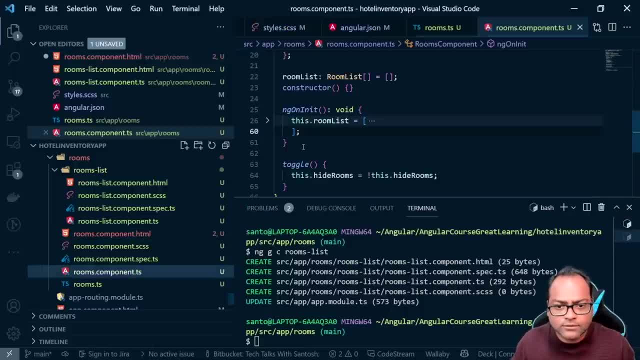 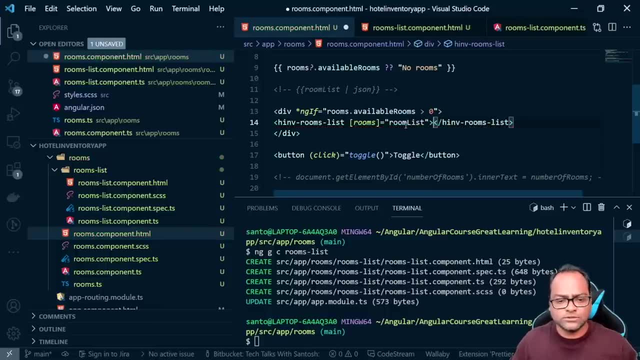 here is called rooms, room list, and we can close this html tag. so, and we can close this html tag so, and we can close this html tag. so this is it now. let's save this and see this. is it now? let's save this and see this. is it now? let's save this and see if it is already compiled, because our 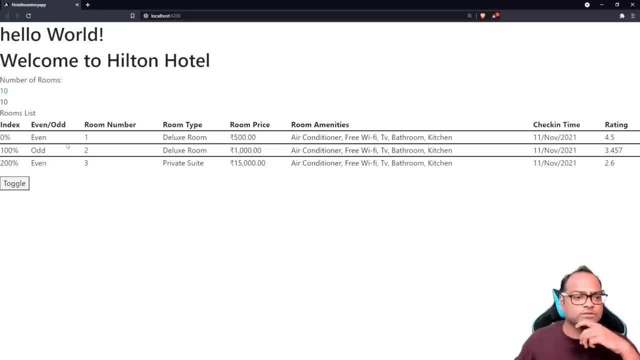 if it is already compiled because our. if it is already compiled because our application is, application is application is really small, and see here so you can see really small, and see here so you can see really small, and see here so you can see. okay, now you have your entire data. 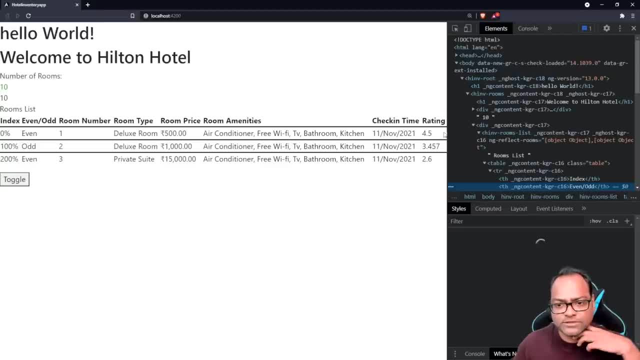 okay, now you have your entire data. okay, now you have your entire data available. but let's verify if it's true, available. but let's verify if it's true, available, but let's verify if it's true, right, i mean if it's actually coming right, i mean if it's actually coming. 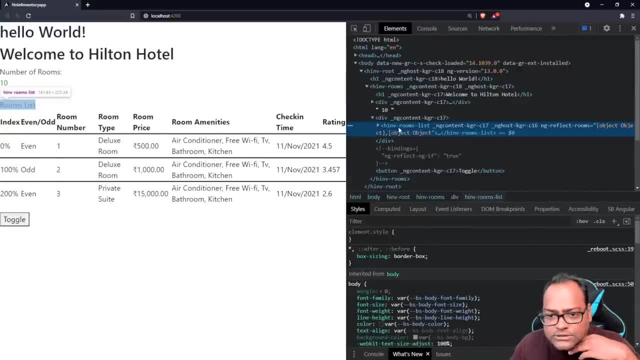 right, i mean, if it's actually coming from the rooms list and you can see from the rooms list and you can see from the rooms list and you can see here. so this is your hotel inventory here. so this is your hotel inventory here. so this is your hotel inventory management and hyphen rooms list. this. 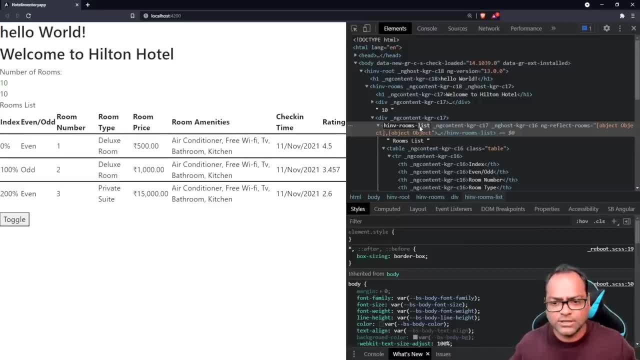 management and hyphen rooms list. this management and hyphen rooms list, this is the new html tag which we created. but is the new html tag which we created. but is the new html tag which we created. but where is this is gone? let's go ahead. where is this is gone? let's go ahead. 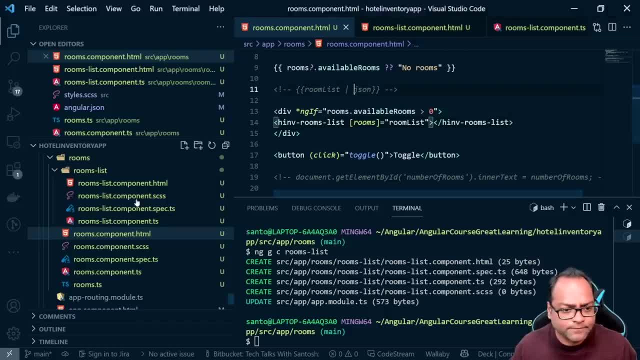 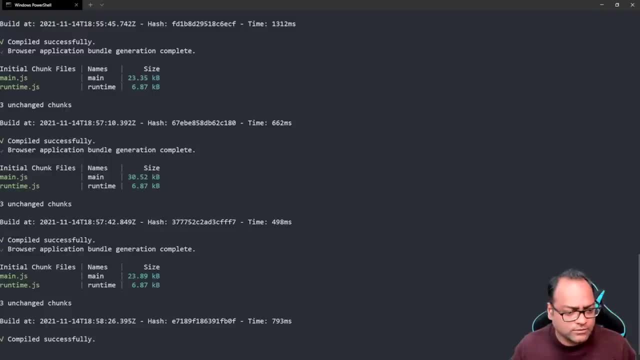 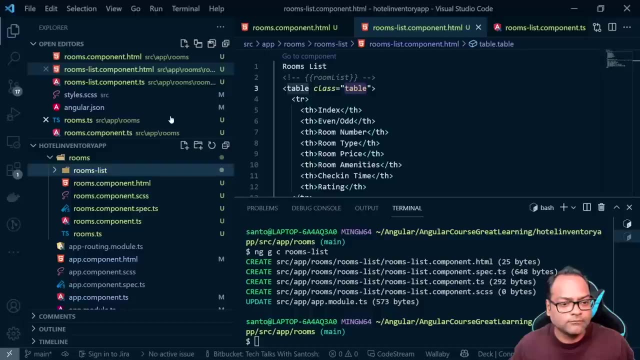 where is this is gone? let's go ahead and try to see that. and we have rooms class table. okay, sorry, if you remember we had added. okay, sorry, if you remember we had added. okay, sorry, if you remember we had added: add odd or even add odd or even. 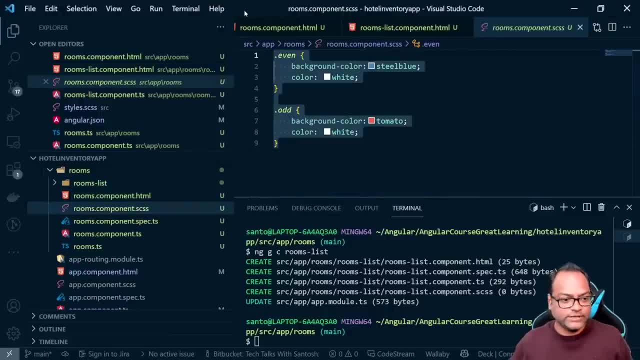 add odd or even style. so you can see odd and even is style. so you can see odd and even is style. so you can see odd and even is actually added here. so it is part of actually added here. so it is part of actually added here, so it is part of room component. how is this happening? we 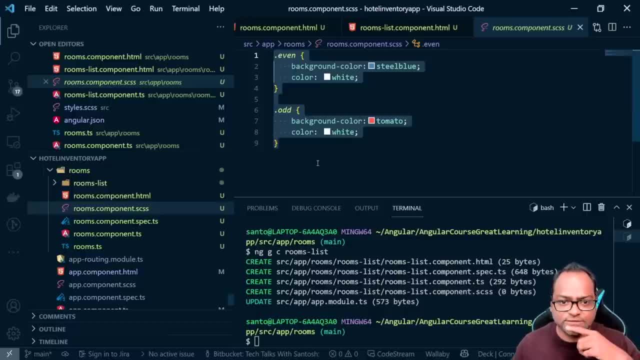 room component. how is this happening? we room component. how is this happening? we will talk about it. there is, there is- will talk about it. there is, there is, will talk about it. there is. there is something called encapsulation which we, something called encapsulation which we, something called encapsulation which we need to talk about. 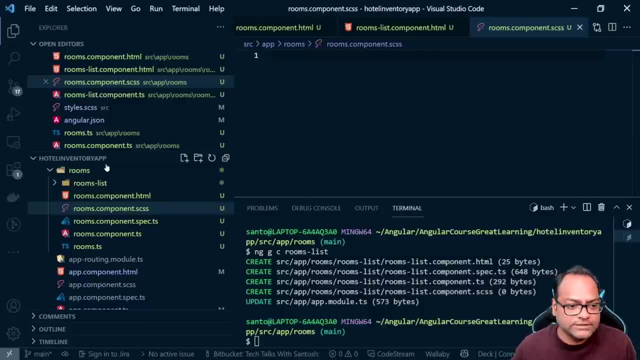 need to talk about. need to talk about currently what we can do. is you we can currently what we can do? is you we can currently what we can do? is you we can actually add it inside rooms list, or actually add it inside rooms list, or actually add it inside rooms list, or we can add. 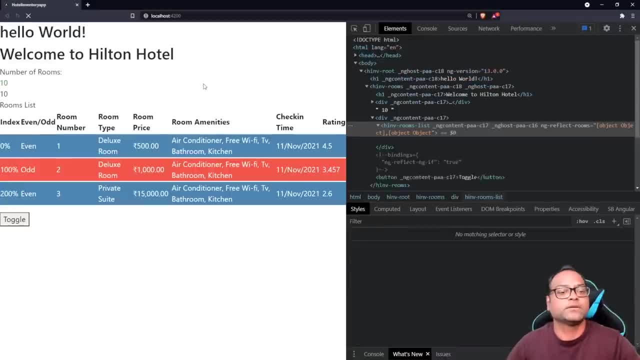 we can add, we can add in our global styleship. so let's do that in our global styleship, so let's do that in our global styleship. so let's do that. and once it is added in global, it is. and once it is added in global, it is. 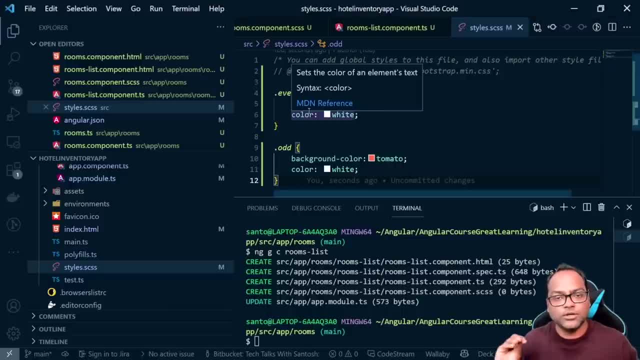 and once it is added in global, it is available. so available, so available. so that's that's it. that's this is how that's that's it. that's this is how that's that's it. that's this is how you're you can pass input to your. 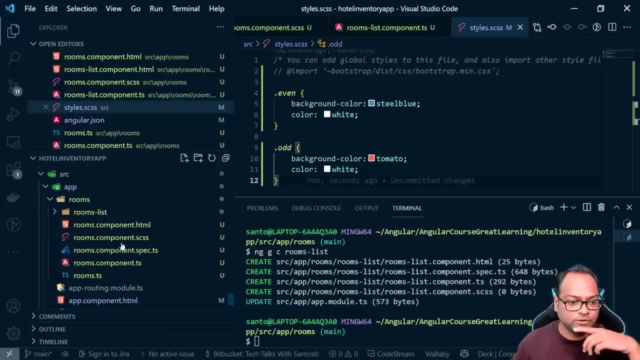 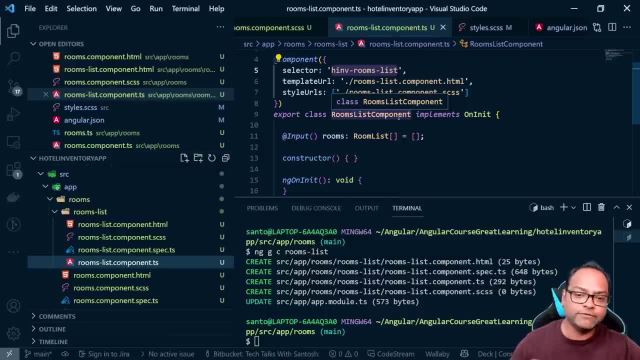 you're, you can pass input to your you're, you can pass input to your component. now what we made it, what we component now, what we made it, what we component now, what we made it, what we made possible right now. so if you think made possible right now, so if you think, 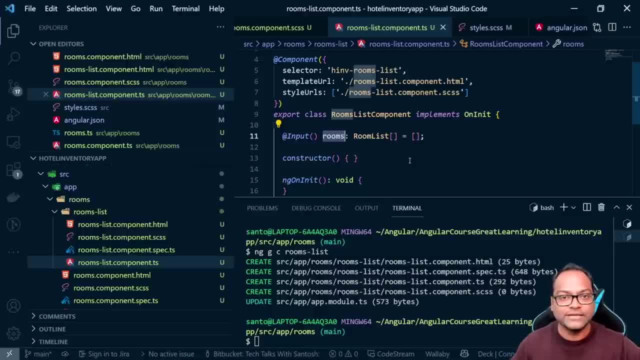 made possible right now. so if you think this property to this particular, this property to this particular, this property to this particular component, so i'm not restricted to use component, so i'm not restricted to use component, so i'm not restricted to use this component only at certain places, i 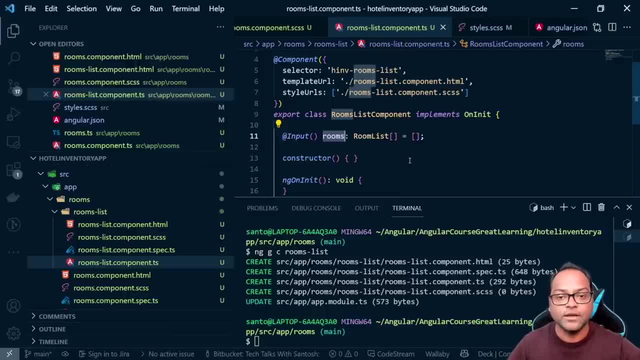 this component only at certain places. i this component only at certain places. i can use it anywhere. i want because this can use it anywhere. i want because this can use it anywhere. i want because this rooms component, rooms component, rooms component- only contains information about how to, only contains information about how to. 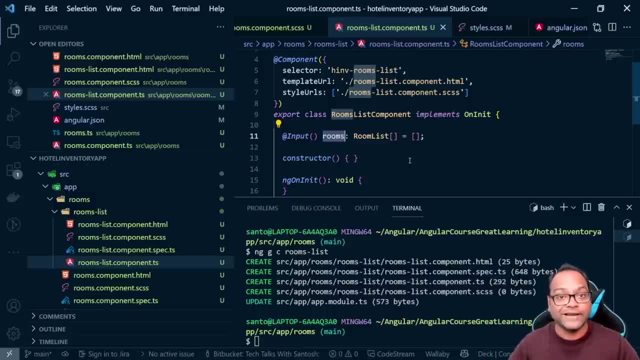 only contains information about how to render things, not how to get the data or render things. not how to get the data or render things, not how to get the data or how to retrieve the data. how to retrieve the data, how to retrieve the data in real world application. we call this. 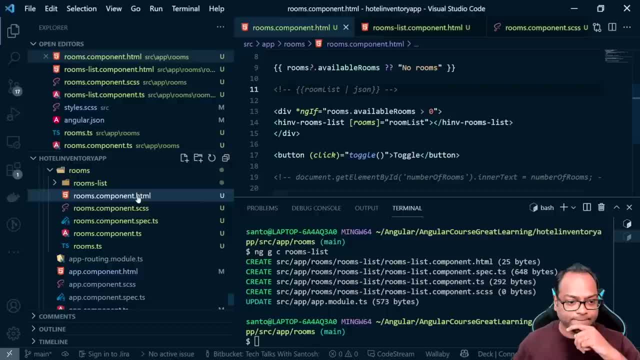 in real world application. we call this in real world application. we call this relationship between relationship, between relationship between these two components, these two components, these two components: rooms component and rooms list rooms component and rooms. list rooms component and rooms. list component as parent and child component: as parent and child. 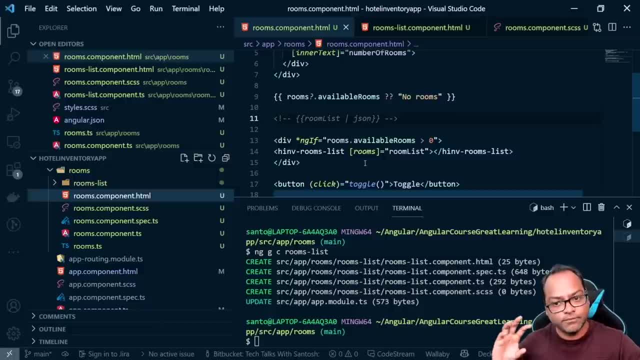 component as parent and child. you can also call this relationship as you can also call this relationship, as you can also call this relationship as smart component, dumb component. so this smart component, dumb component. so this smart component, dumb component. so this is for smart component which knows, is for smart component which knows. 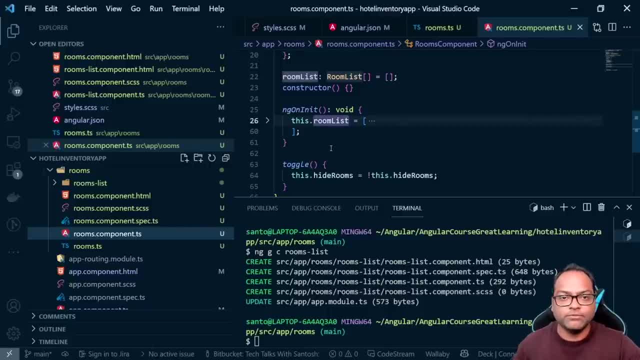 is for smart component which knows from where to get the data, from where to get the data, from where to get the data, and some and some and some. some action which needs to be performed, some action which needs to be performed, some action which needs to be performed. and this is your dumb component which 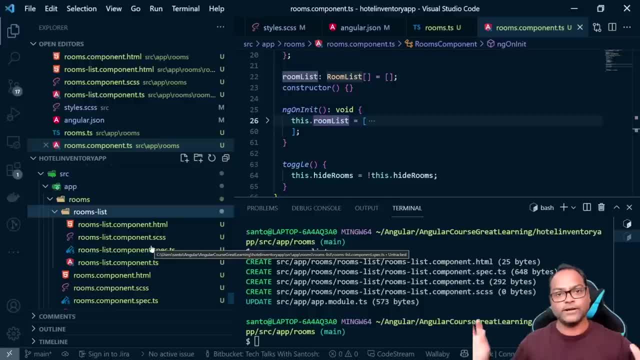 and this is your dumb component which- and this is your dumb component- which doesn't know anything. it just needs to. doesn't know anything. it just needs to. doesn't know anything. it just needs to know how what to render. that's it. know how what to render, that's it. 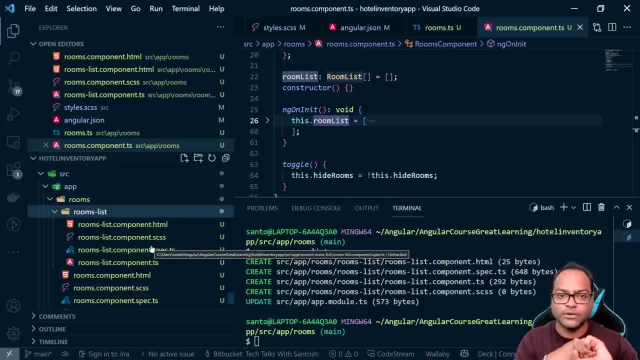 know how, what to render that's it so parent child, so parent child, so parent child. smart component- uh dumb component. these smart component- uh dumb component. these smart component- uh dumb component. these are the things which you are, the things which you are, the things which you uh. 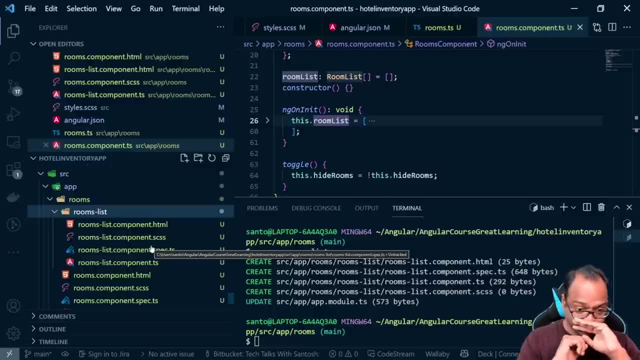 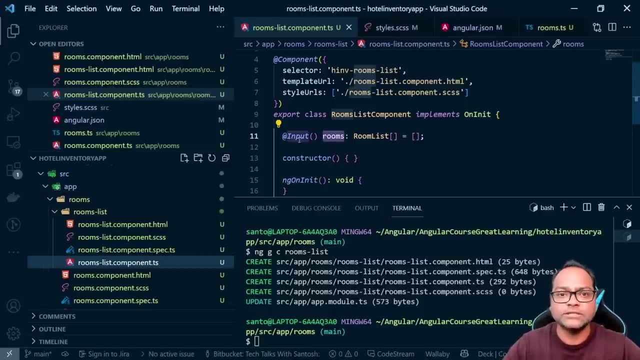 uh, uh. if you come across these things, this is if you come across these things, this is if you come across these things, this is what you mean in your real-time enterprise application, in your real-time enterprise application, in your real-time enterprise application, try to split your components to. 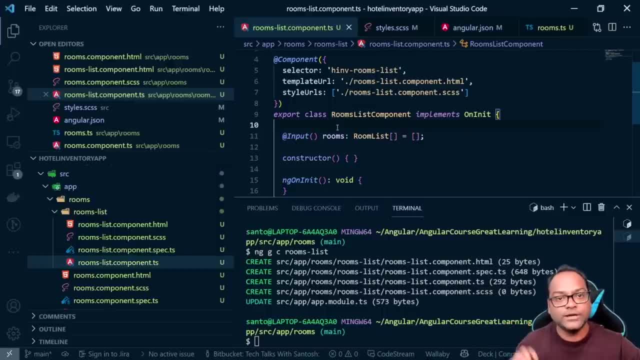 try to split your components. to try to split your components to as smallest level as possible. as smallest level as possible, as smallest level as possible. don't have a component with like. don't have a component with like. don't have a component with like. thousands of html or thousand slice. 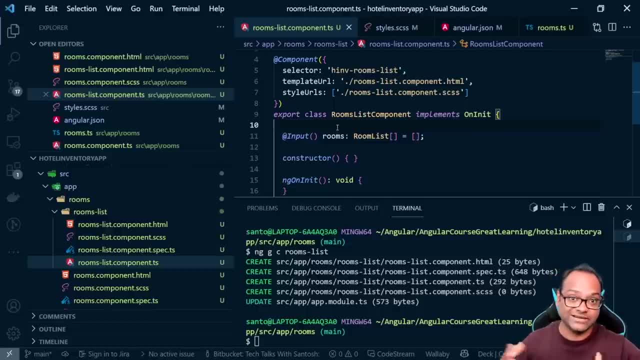 thousands of html or thousand slice thousands of html or thousand slice lines of ts. try to split them as much lines of ts. try to split them as much lines of ts. try to split them as much as possible, generalize them as possible. generalize them as possible, generalize them and, uh, try to have like small component. 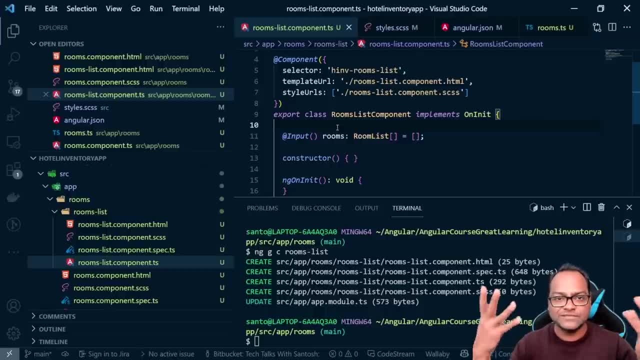 and uh, try to have like small component and uh, try to have like small component for each logic, for each logic, for each logic. so here we knew that, okay, there is a. so here we knew that. okay, there is a. so here we knew that. okay, there is a rooms list which needs to be created. so 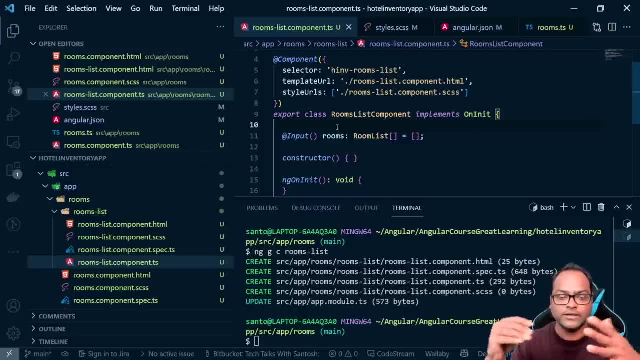 rooms list which needs to be created, so rooms list which needs to be created. so what we did is we created. what we did is we created another room rooms list component, which another room rooms list component, which another room rooms list component which will take care of rendering those things. 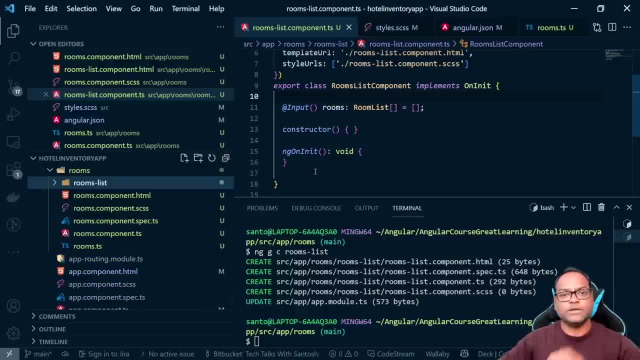 will take care of rendering those things, will take care of rendering those things now, now, now in real-time application. now let's, let's in real-time application, now let's, let's in real-time application. now let's, let's talk about the term right smart. talk about the term right smart. 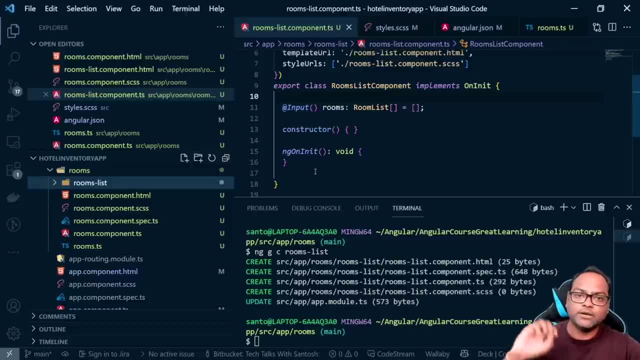 talk about the term right: smart component, dumb component component, dumb component component, dumb component- in real-time applications. now your in real-time applications, now your in real-time applications. now your child component may need to. child component may need to. child component may need to do some action. 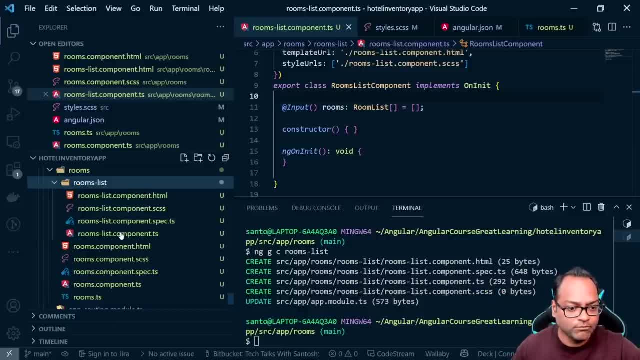 do some action. do some action, for example. so let's say, uh, we want to, for example. so let's say, uh, we want to, for example. so let's say, uh, we want to actually actually actually, we have this rooms list, now i want to. we have this rooms list, now i want to. 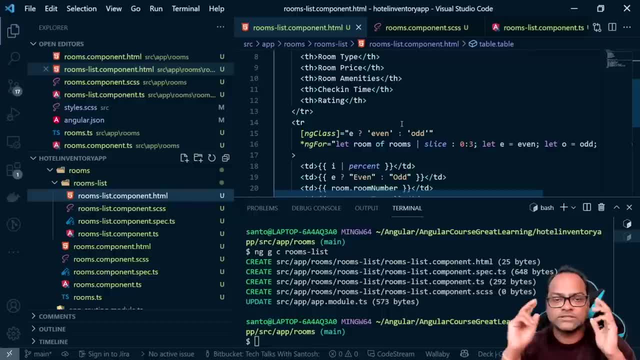 we have this rooms list. now i want to give an action button at the end. and i give an action button at the end and i give an action button at the end and i want to say, want to say, want to say: book this room or uh, book this room or uh. 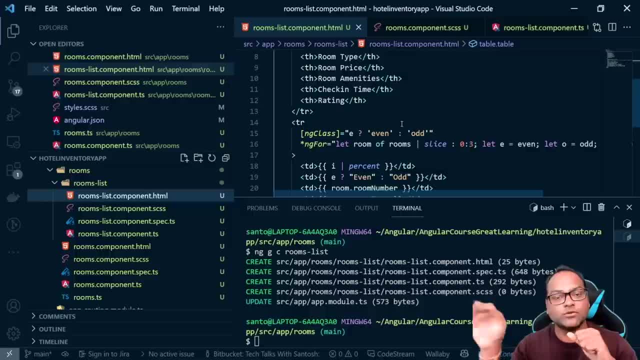 book this room, or uh marks it, mark it as sold right. so this marks it, mark it as sold right, so this marks it, mark it as sold right. so this is something. uh, so this hotel becomes is something. uh, so this hotel becomes is something uh, so this hotel becomes not available. 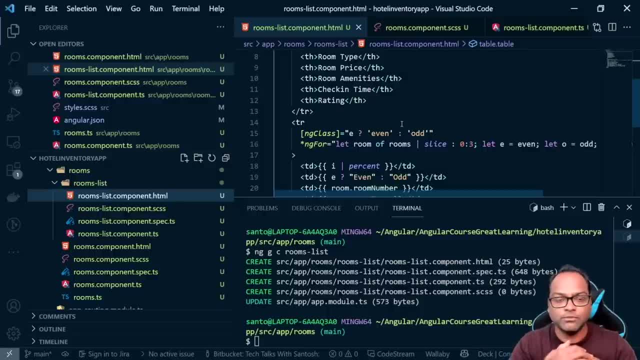 not available. not available. we are saying this particular component, we are saying this particular component. we are saying this particular component is child component or dumb component. so is child component or dumb component. so is child component or dumb component. so it cannot take action on its own. it cannot take action on its own. 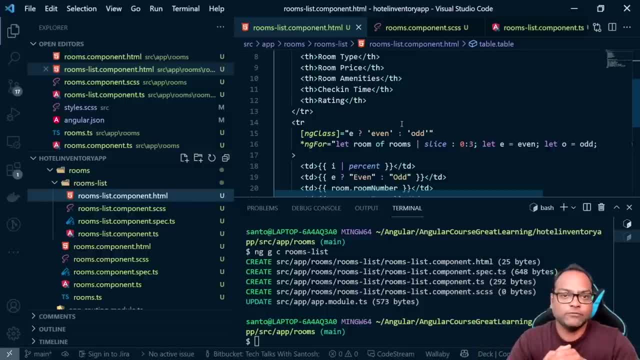 it cannot take action on its own. simple example, real-time scenario of simple example. real-time scenario of simple example. real-time scenario, of course, if you have a kid course, if you have a kid course, if you have a kid, what you, what kids do? right, they come to. 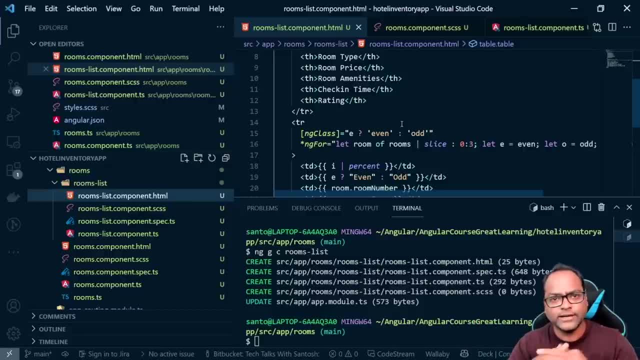 what you, what kids do right. they come to what you, what kids do, right. they come to you and say okay, you. and say okay, you. and say okay, i need this thing, and then you do it, i need this thing, and then you do it, i need this thing. and then you do it right and you don't give money to your 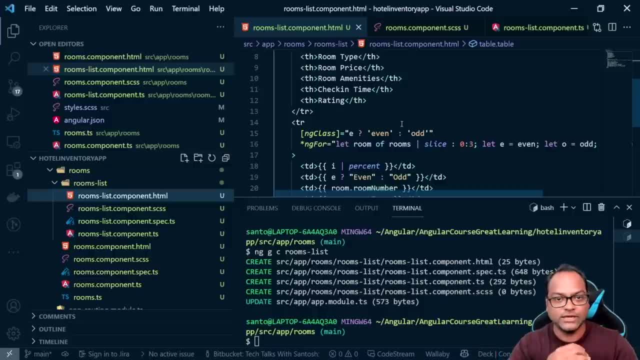 right and you don't give money to your right and you don't give money to your kid and say kid, and say kid and say good invite until of course they, they good invite, until of course they, they good invite, until of course they, they became, became, became they, they become smart, right, i mean they. 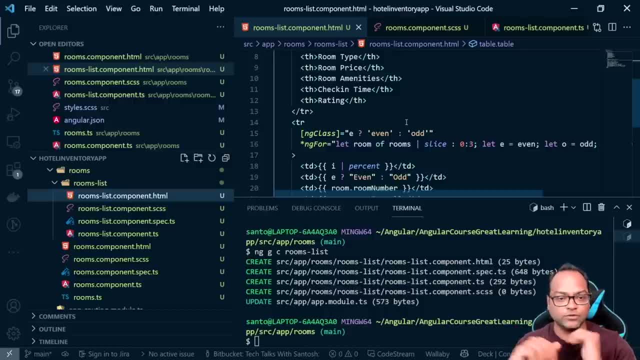 they, they become smart, right, i mean they, they, they become smart, right. i mean they know how to deal with things. know how to deal with things. know how to deal with things. so same same concept is applied here. so so same same concept is applied here. so so same same concept is applied here. so now, as my child component, or my dumb, 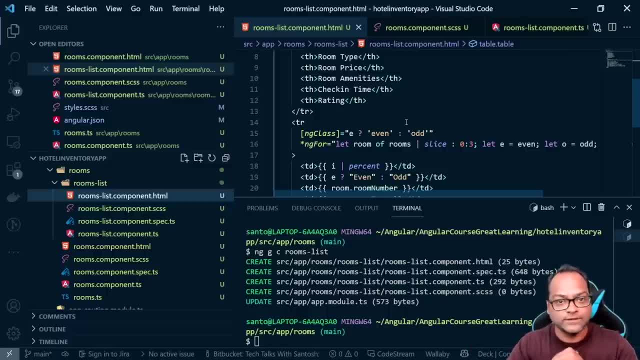 now as my child component, or my dumb now as my child component or my dumb component. doesn't know component doesn't know component doesn't know or doesn't need to know how to do stuff. or doesn't need to know how to do stuff or doesn't need to know how to do stuff, what it can do. 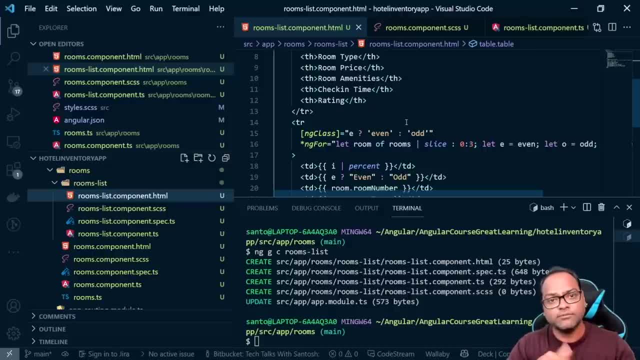 what it can do, what it can do in case it needs to perform some action, in case it needs to perform some action. in case it needs to perform some action, it can ask. it can ask parent, it can ask the smart component. parent, it can ask the smart component. 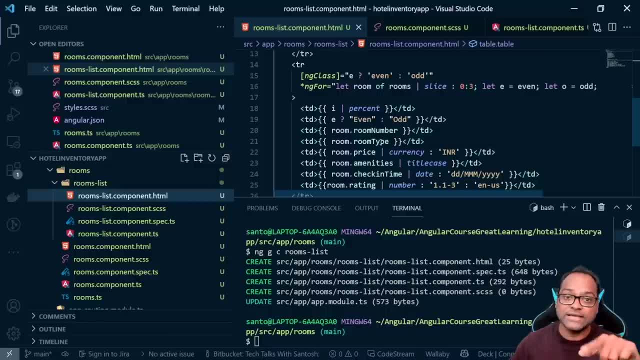 parent. it can ask the smart component to do stuff, to do stuff. to do stuff. this is where we need to pass the data. this is where we need to pass the data. this is where we need to pass the data back from child to parent component, back from child to parent component. 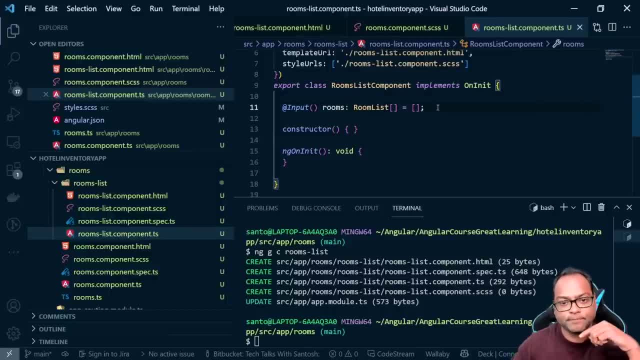 back from child to parent component. how to achieve that? of course output right. so we are saying: of course output right. so we are saying: of course output right. so we are saying: input can get the data output. can input can get the data output. can input can get the data output can give out the data. so let's create an. 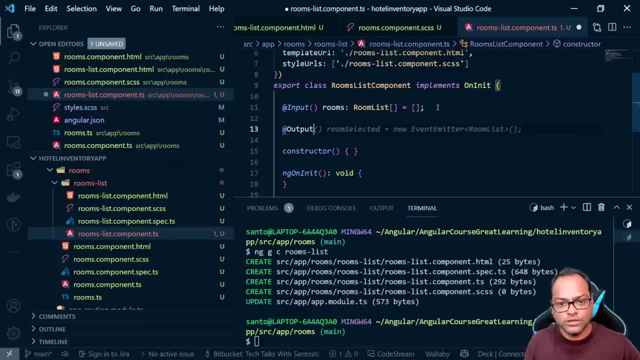 give out the data, so let's create an. give out the data, so let's create an output: output, output and outputs are actually an event, so, and outputs are actually an event, so, and outputs are actually an event, so let's right now, let's create an event. 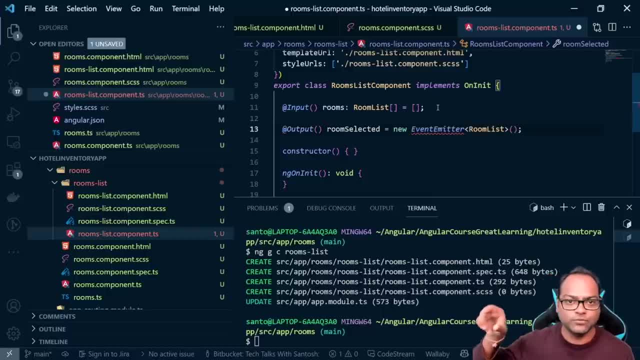 let's, right now, let's create an event. let's, right now, let's create an event called, called, called, room selected. so i we will click on room selected, so i we will click on room selected, so i we will click on this room, this room, this room, we'll say okay, select this room. and 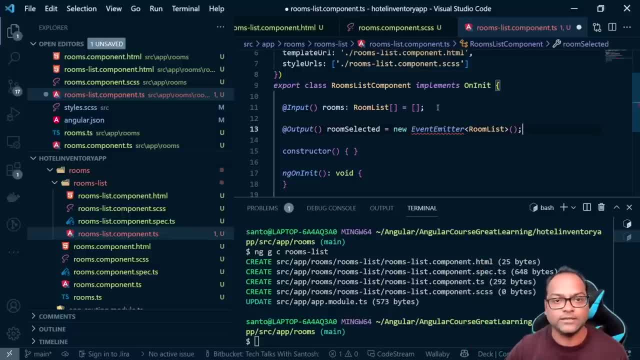 we'll say, okay, select this room. and we'll say, okay, select this room, and this information will be passed to your. this information will be passed to your. this information will be passed to your parent and your parent can do anything. parent and your parent can do anything. 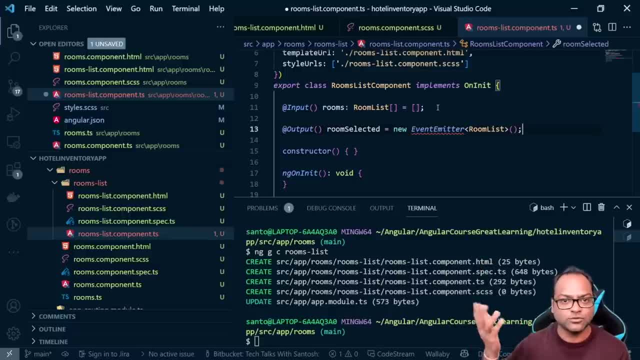 parent and your parent can do anything, whether this room needs to be worked, whether this room needs to be worked, whether this room needs to be worked, this room needs to be marked as sold. this room needs to be marked as sold, this room needs to be deleted, right, i mean? 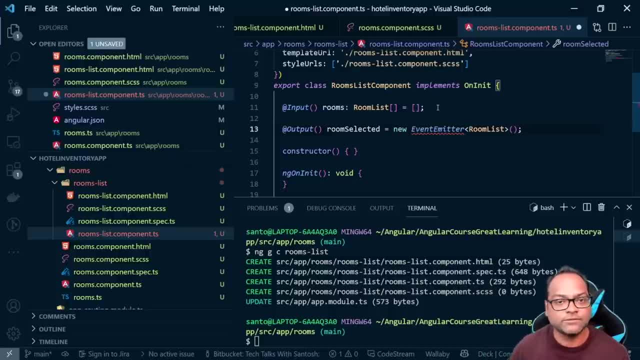 this room needs to be deleted, right. i mean this room needs to be deleted, right. i mean let's say uh. let's say uh, let's say uh. now this room is used for some other. now this room is used for some other. now this room is used for some other purpose. so this room is not available. 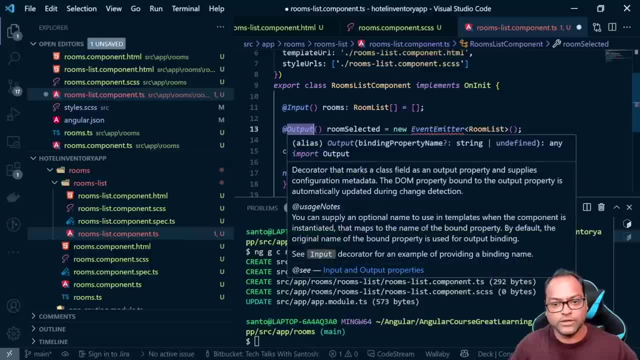 purpose, so this room is not available. purpose, so this room is not available anymore. so what we will do is we'll anymore. so what we will do is we'll anymore. so what we will do is we'll create an output. create an output. create an output decorator. we will use an output. 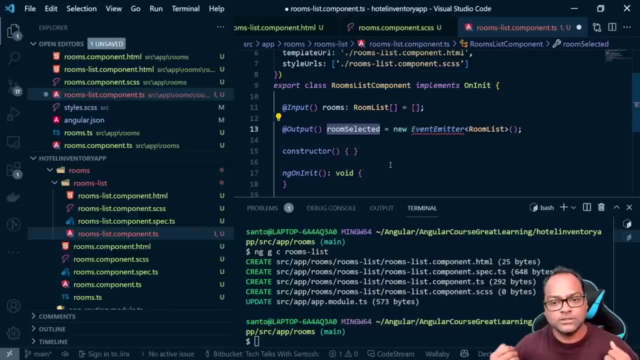 decorator. we will use an output decorator, we will use an output decorator, and then we are saying decorator, and then we are saying decorator, and then we are saying the event name is rooms- room selected. the event name is rooms- room selected. the event name is rooms- room selected, or we can say selected. 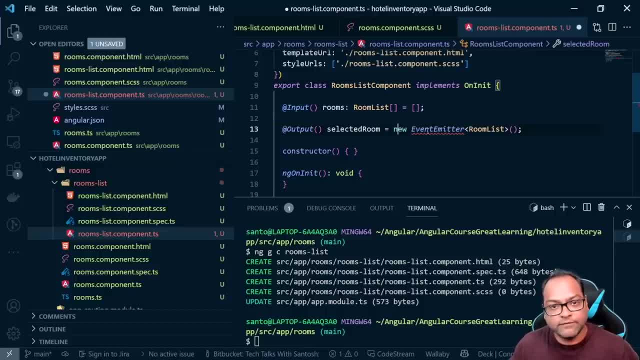 or we can say selected, or we can say selected room, room, room and, and, and it it needs to be an event. so there is a it it needs to be an event. so there is a it it needs to be an event. so there is a new uh event emitter class, which is uh. 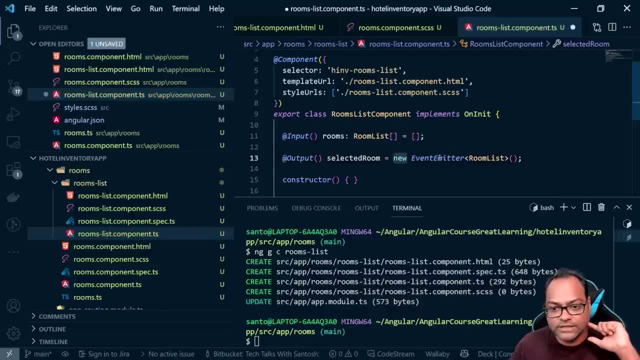 new uh event emitter class which is uh. new uh event emitter class which is uh. available in angular core. available in angular core, available in angular core. which needs to be imported. so we can say which needs to be imported. so we can say which needs to be imported, so we can say new event emitter. and then we have to. 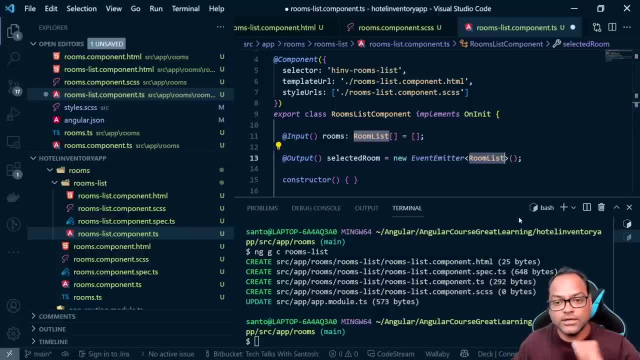 new event emitter and then we have to new event emitter and then we have to tell what kind of data we want to send, tell what kind of data we want to send, tell what kind of data we want to send back to parent. so here the kind of data. 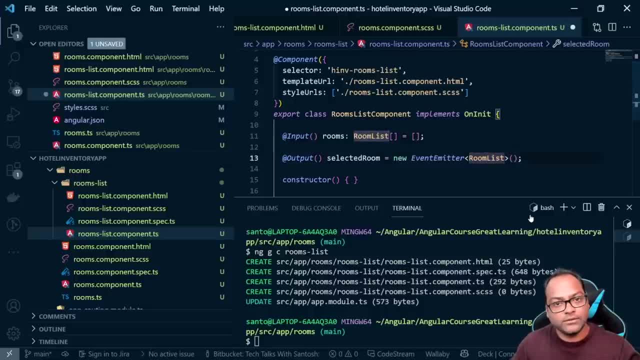 back to parent. so here the kind of data back to parent. so here the kind of data we have is room list. we have is room list. we have is room list. if, if, if it needs to be multiple, of course you can. it needs to be multiple, of course you can. 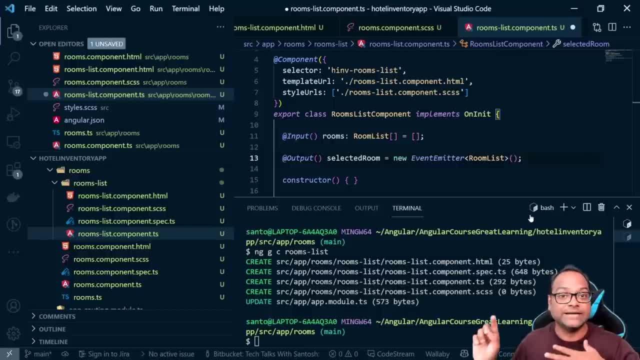 it needs to be multiple. of course, you can put an array, but right now i want to put an array, but right now i want to put an array, but right now i want to just select, just select, just select. send the selected room. so done here. so now, what we will do is we: 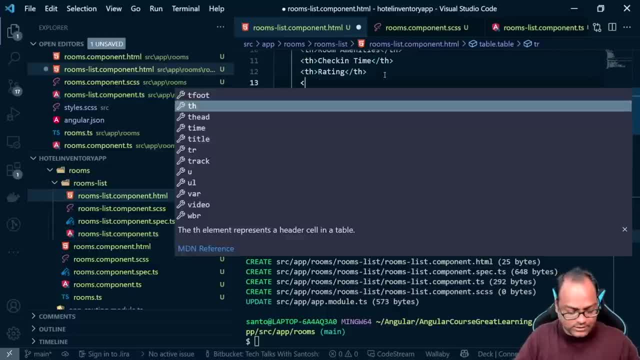 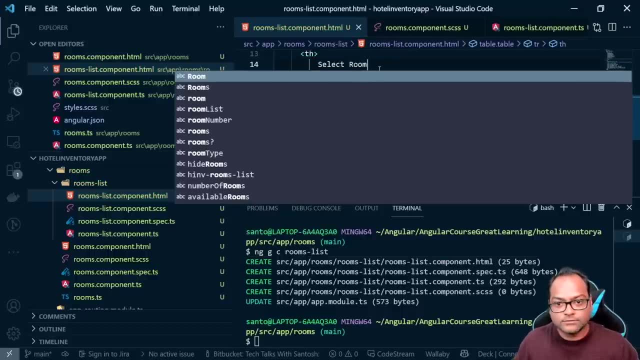 so done here. so now what we will do, is we so done here? so now what we will do is we will add an action here and will add an action here and will add an action here, and i'll create a header and i'll say this: i'll create a header and i'll say: this is select room. 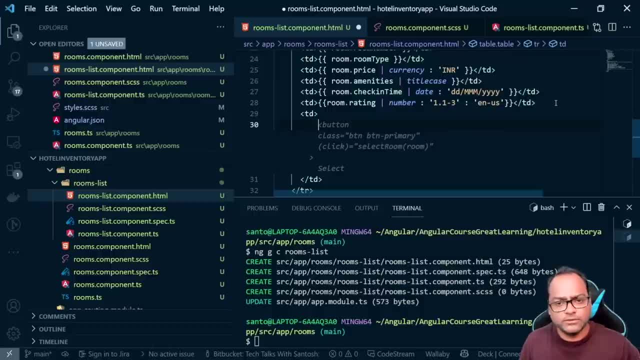 and inside td we will add a button. and inside td we will add a button, and inside td we will add a button. and that's how to complete, so you can say: and that's how to complete, so you can say: and that's how to complete, so you can say: button. 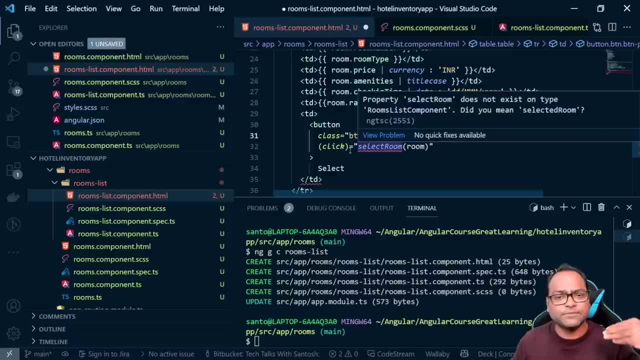 button button class. and btn btn primary is a class and btn btn primary is a class and btn btn primary is a, is a bootstrap class and is a bootstrap class and is a bootstrap class, and this is the function which will. this is the function which will. this is the function which will implement select room. so let's go ahead. 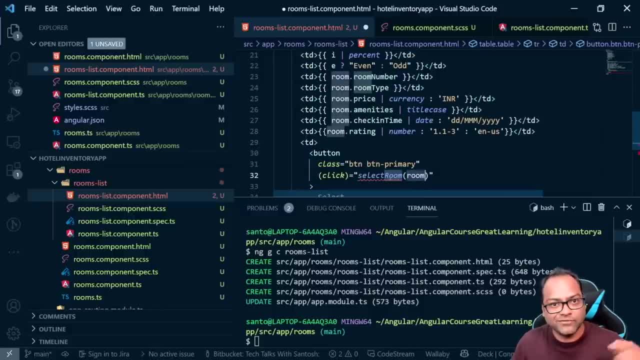 implement select room. so let's go ahead, implement select room. so let's go ahead and see, and this is the room object and this is the room object and this is the room object which we, which it will get once, we, which we which it will get once we. 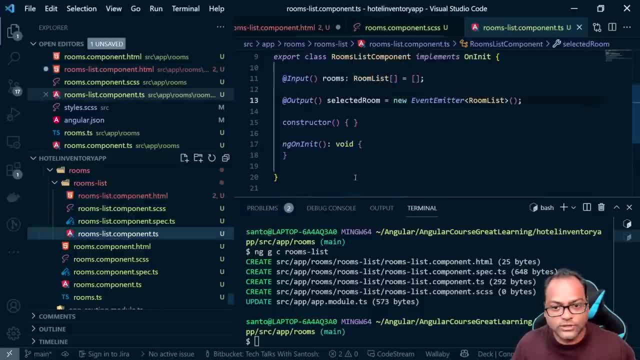 which we, which it will get once we click on this particular room, click on this particular room, click on this particular room. so let's go back to typescript and add. so let's go back to typescript and add. so let's go back to typescript and add this function which is supposed to get. 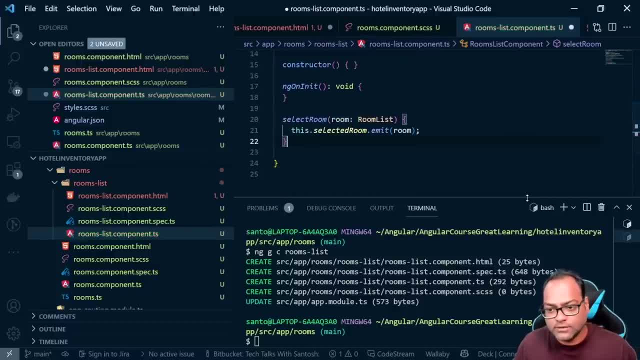 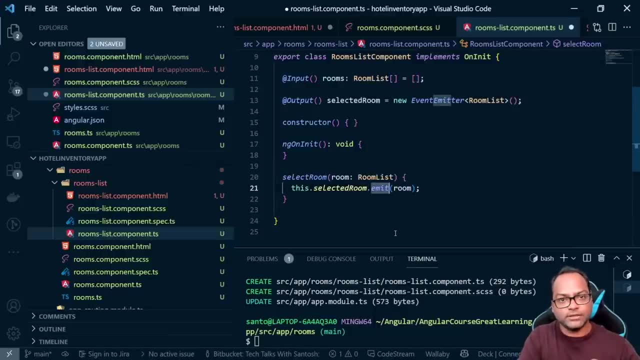 which is supposed to get a room list and which is supposed to get a room list and which is supposed to get a room list, and then once, then, once, then, once this room list or the room is selected, this room list or the room is selected, this room list or the room is selected, we want to emit this data back to parent. 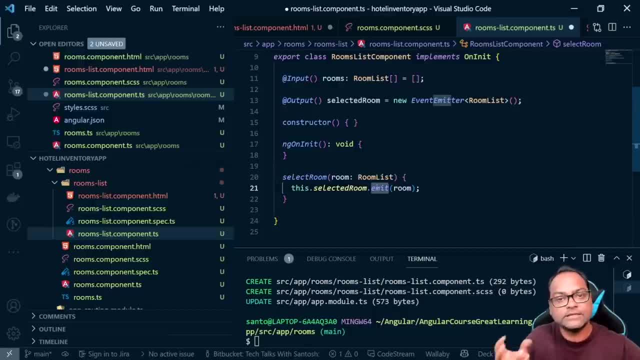 we want to emit this data back to parent. we want to emit this data back to parent. so this, this line of code: selected room. so this, this line of code: selected room. so this, this line of code: selected room. dot emit will give this data back to. dot emit will give this data back to. 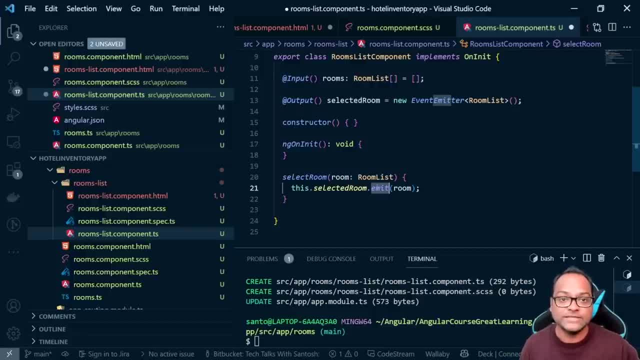 dot emit will give this data back to the parent. who has the parent, who has the parent, who has. remember who has actually uh subscribed. remember who has actually uh subscribed. remember who has actually uh subscribed to this event. it's not something like i to this event. it's not something like i. 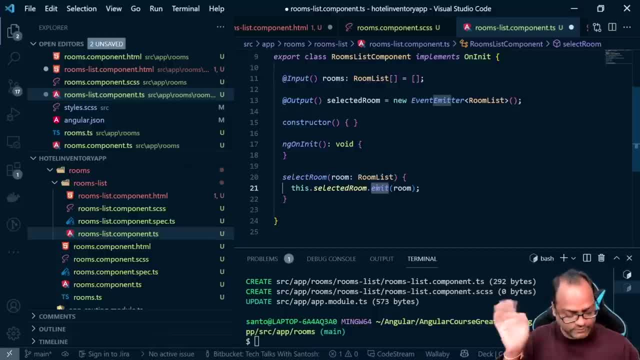 to this event. it's not something like i mean, if i'm not uh subscribing to this, mean, if i'm not uh subscribing to this mean, if i'm not uh subscribing to this event, this won't be available, so let's event. this won't be available, so let's. 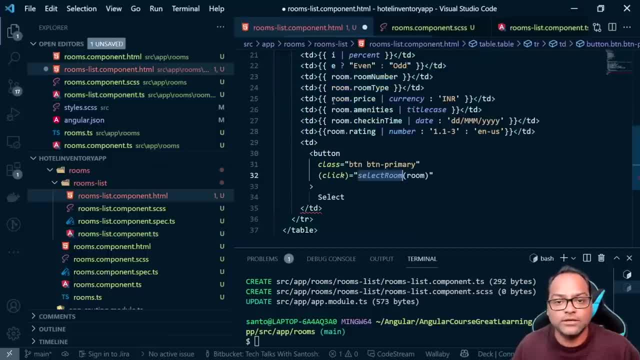 event. this won't be available. so let's go ahead and see that part of us see. go ahead and see that part of us see, go ahead and see that part of us see that part of the code. so here, this is that part of the code. so here this is. 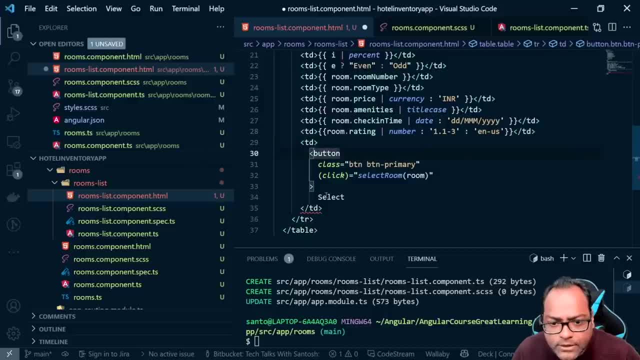 that part of the code. so here this is our uh okay, our uh okay, our uh okay button. it was not closed, so it was not closed, so it was not closed. so now let's go back to the parent, which is. now let's go back to the parent, which is: 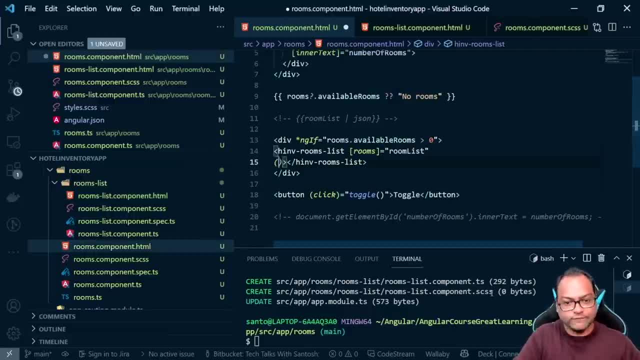 now let's go back to the parent which is this one, this one, this one, and let's implement the event. so we know, and let's implement the event. so we know. and let's implement the event. so we know the name: selected room. this is the event. 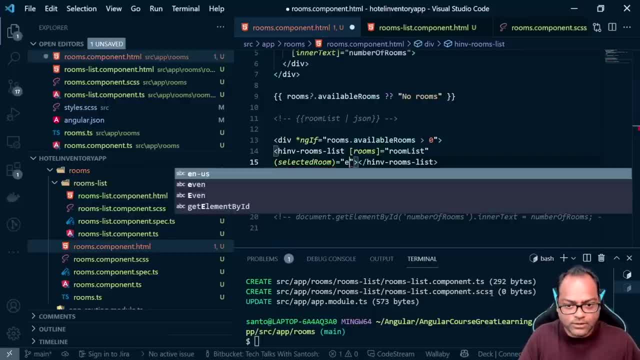 the name selected room. this is the event. the name selected room. this is the event. name, name, name, and i'll and i'll and i'll write a local function which selects the write. a local function which selects the write. a local function which selects the room room. 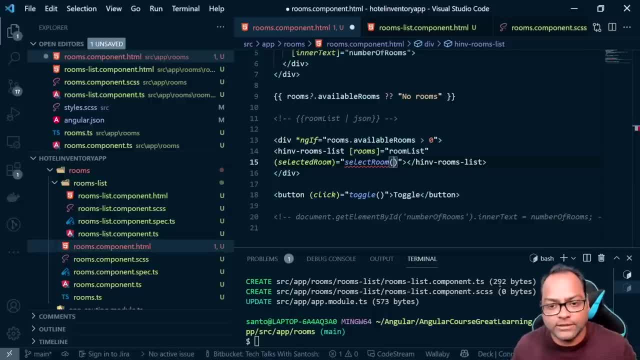 room so we can say select two, so we can say select two, so we can say select two, and this is something which is not and this is something which is not and this is something which is not implemented right now. let's go ahead and implemented right now. let's go ahead and. 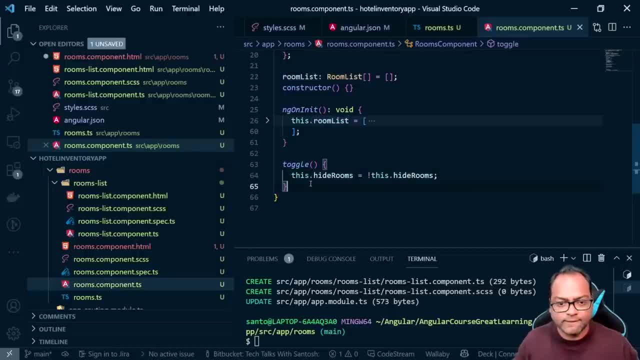 implemented. right now, let's go ahead and implement, implement, implement. so here, what i will do is: uh first, let's. what i will do is uh, first. let's what i will do is uh, first, let's add a consolelog. add a consolelog. add a consolelog so it says: selected room which takes a. 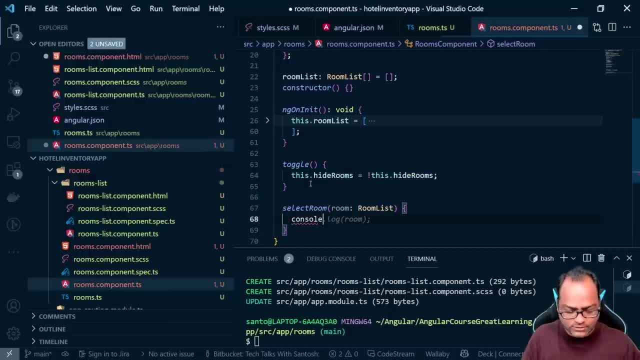 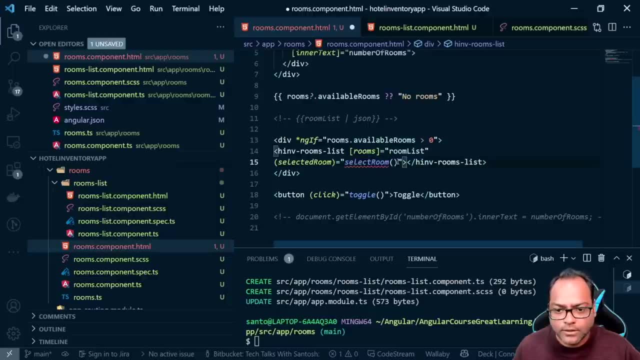 so it says selected room, which takes a. so it says selected room which takes a room and room and room. and we print consolelog room. we print consolelog room. we print consolelog room. save this here now, as we are getting some data. we here now, as we are getting some data. we. 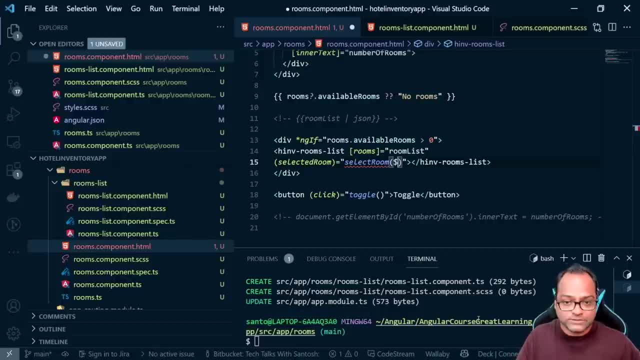 here now, as we are getting some data, we have to actually pass some information, have to actually pass some information, have to actually pass some information here. so here you have to pass something here. so here you have to pass something here. so here you have to pass something called as dollar event. 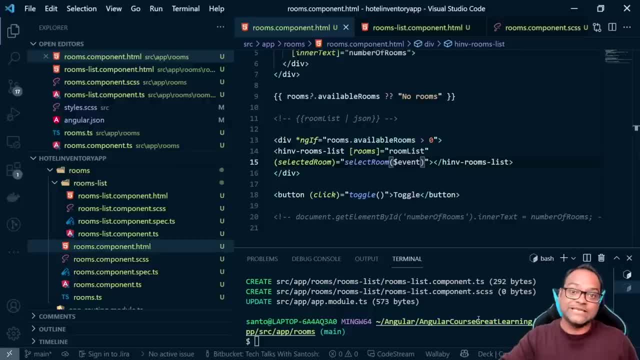 called as dollar event. called as dollar event, this always remains dollar event. so this always remains dollar event. so this always remains dollar event. so this is an event which will be received. this is an event which will be received. this is an event which will be received from my child component. 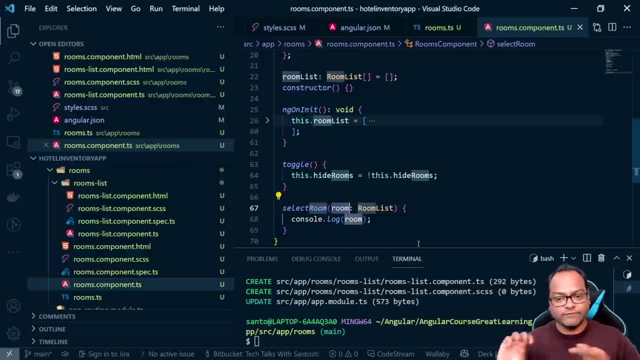 from my child component, from my child component, and here you can specify that: okay, uh, and here you can specify that, okay, uh, and here you can specify that, okay, uh, this event, uh, which will be this event, uh, which will be this event, uh, which will be sending me the data of this type. so 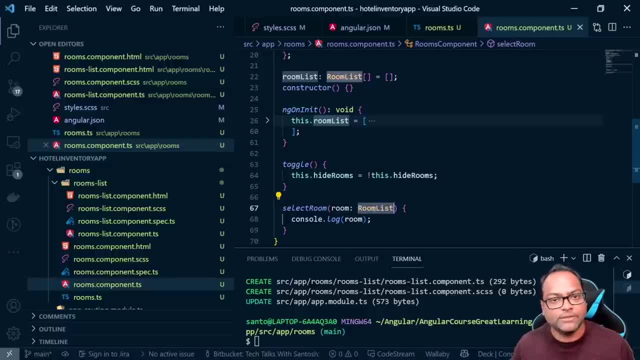 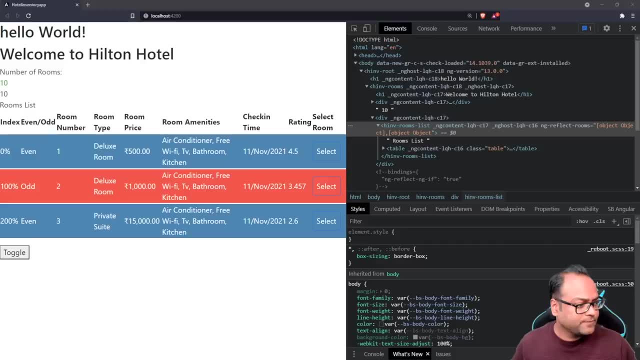 sending me the data of this type. so So this room, sorry, this data will be type of room list. So far, so good. Let's see our build just completed. Let's see our application. Now we have the select button. 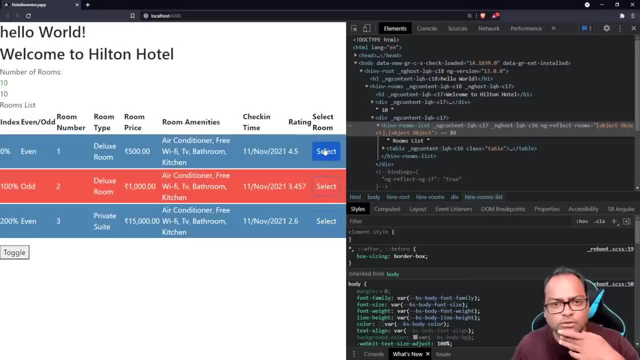 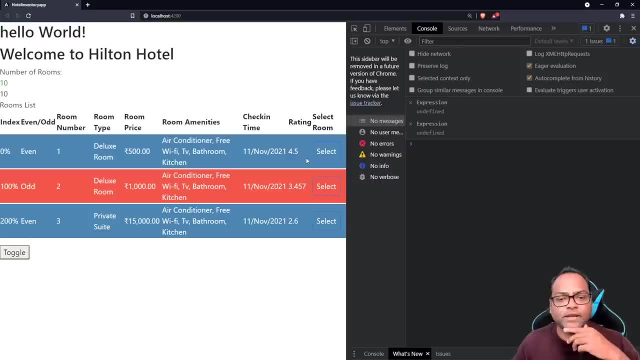 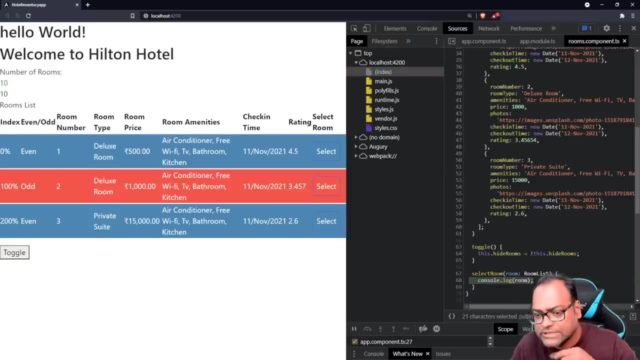 You can see when you hover it becomes blue, right? So let's go to console and let's delete, and let's click on select And you can see. okay, now you have this. rooms componentts, line number 68.. This is where this information is coming, right. 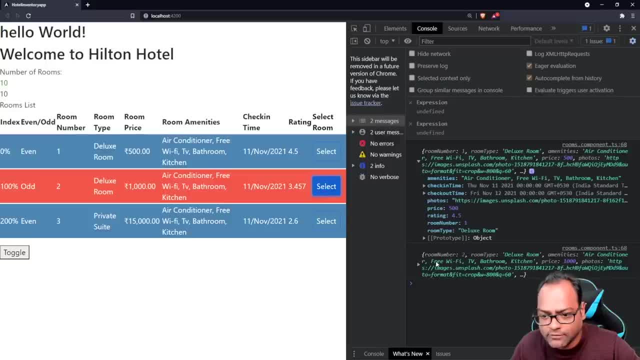 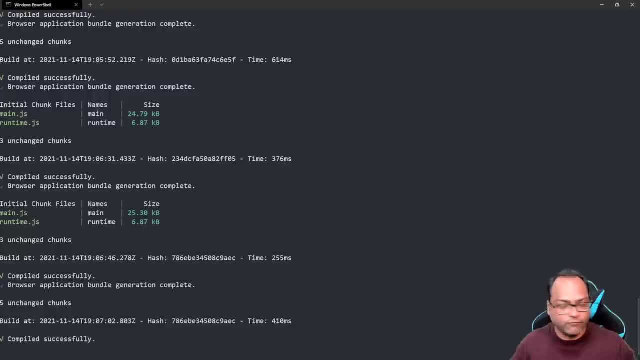 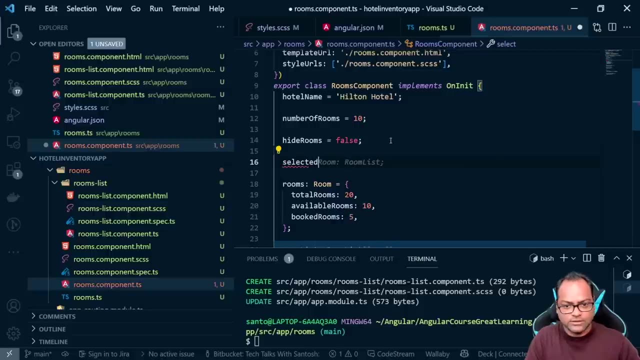 So you have your amenities check-in time, check-out time and whichever row you select, you get that row specific data sent to your parent. So this is how your output works. Now we can actually do something more with this. I can say, okay, this is selected room, which is type of room list. 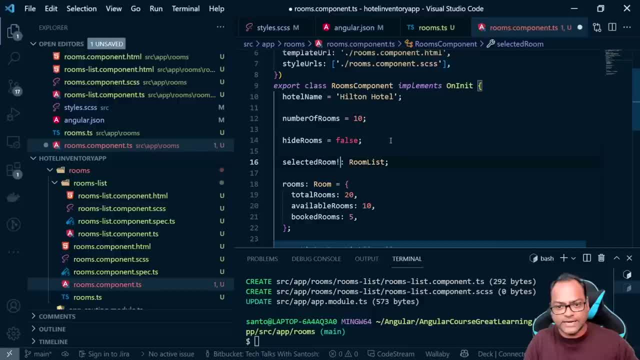 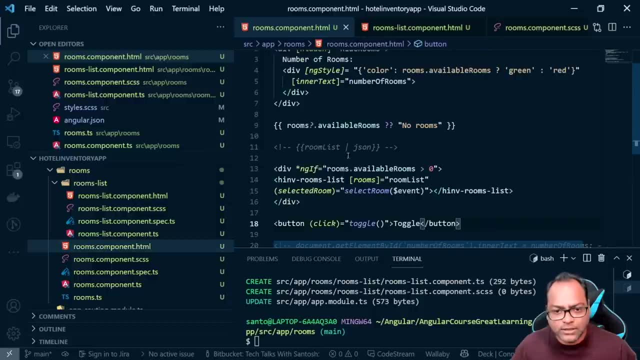 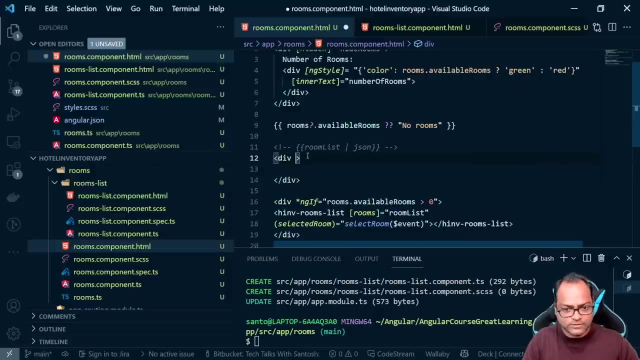 And as we are using strict mode, I'll just add this so we don't get the error. And now here, let's do it just above the table, So I can say this div is and we will use star ng. if So, we'll just display it in case selected rooms exist. 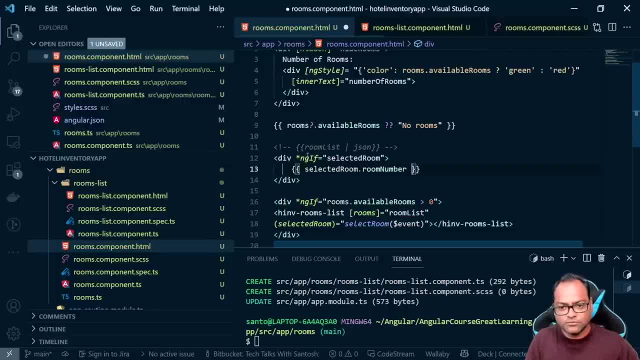 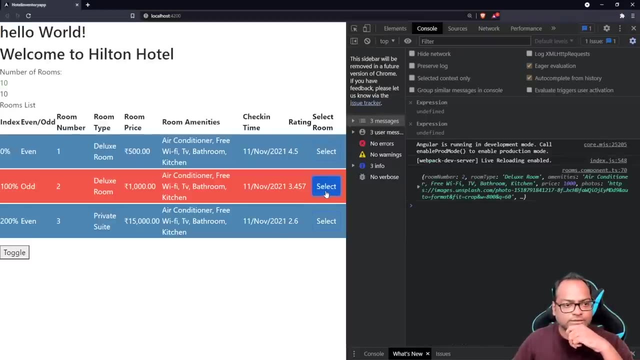 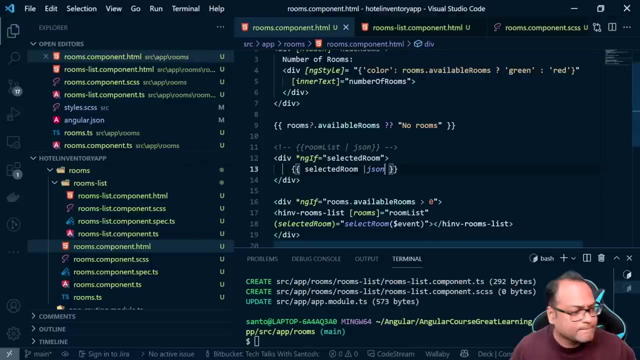 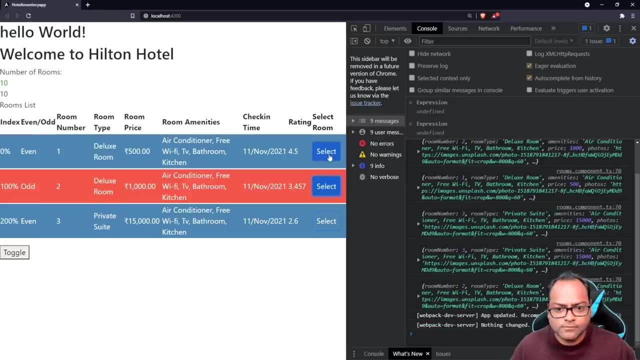 And then we can say, okay, this selected room, or let's use JSON pipe right to see what information we have available. Let's go back and let's click on select, Because there which is not saved looks like We're going to pause and try something again. 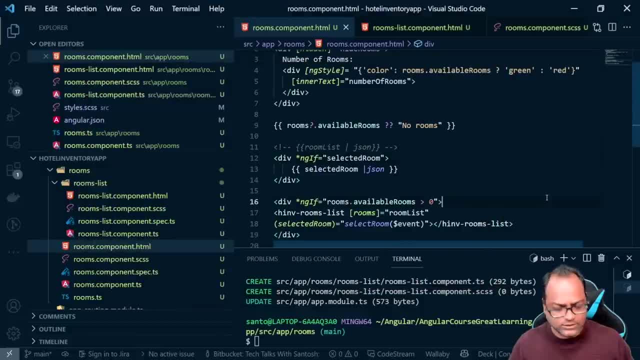 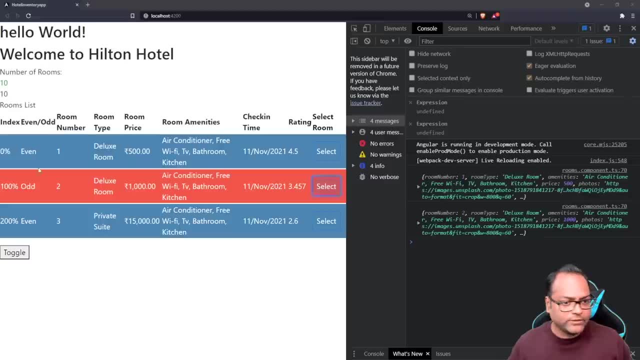 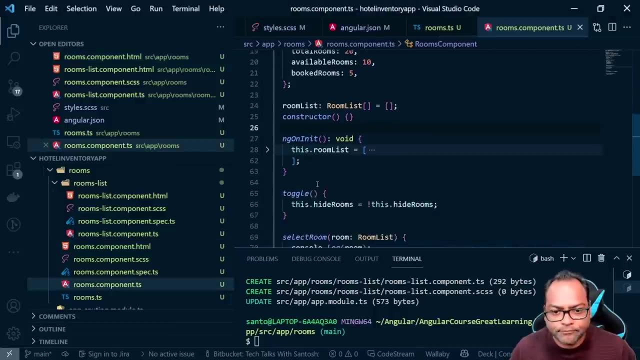 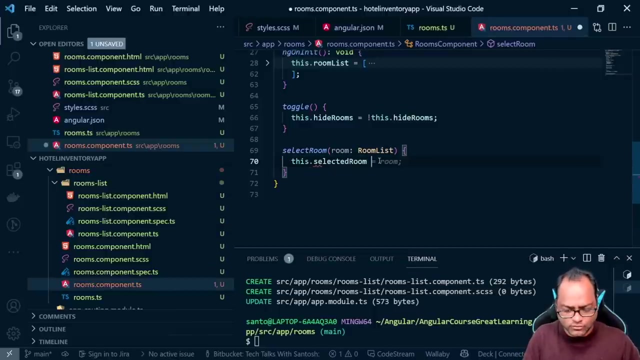 Okay, You're not getting recompiled. okay, it is not. So somehow, not, it is done. Let's click on select. Ah, my bad, So we have to assign this value right. So this dot selected room is equals to: and. once we have assigned this value, now let's. 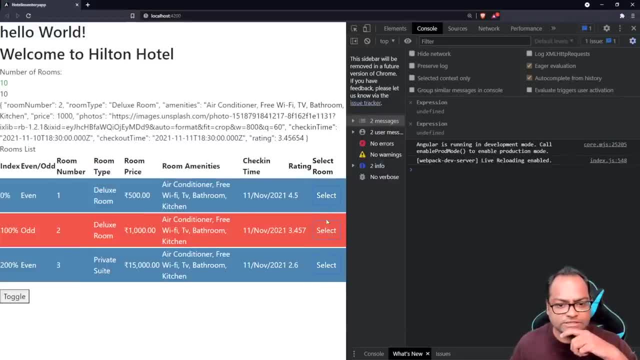 go ahead and click on selected room. You can see the information is getting changed based on what data you emit from your child component. So this is how you can communicate between two components- child and parent, or smart component, dumb component, using input and. 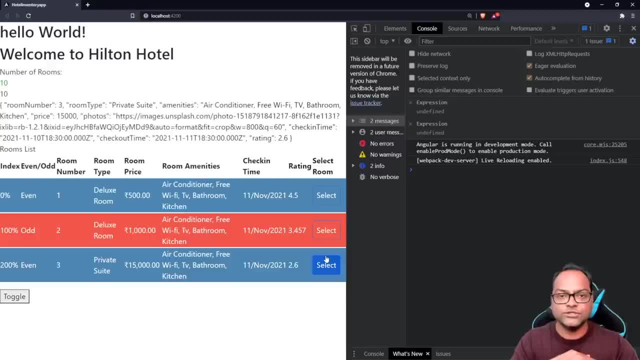 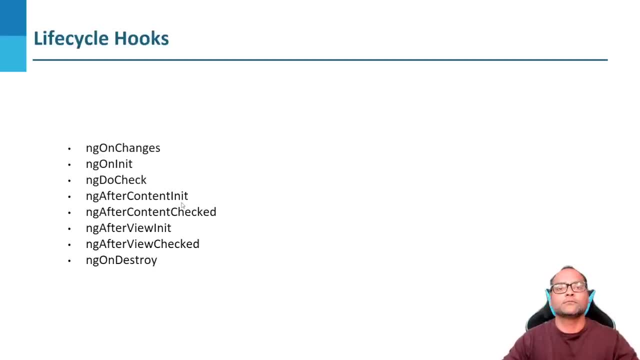 output Now how it is related to ngOnChanges event, because that's why we did this. We'll see that next. So far we have seen the ngOnInit lifecycle look and we also saw how we can do component communication using input and output. And we did that because we wanted 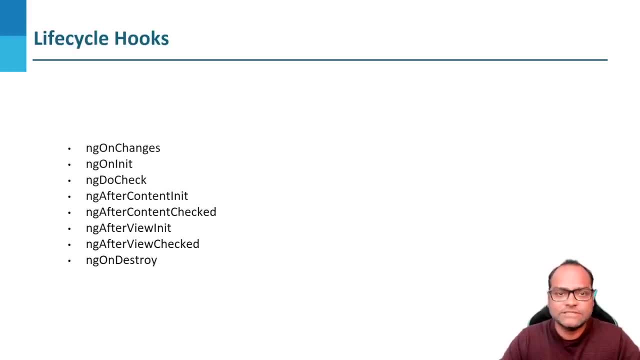 to talk about ngOnChanges lifecycle event. So let's go ahead and do that. And while talking about ngOnChanges, we will also talk about one very important concept, which is known as change detection, And this is like a really important topic, even in interviews as well. A lot of questions may be asked related. 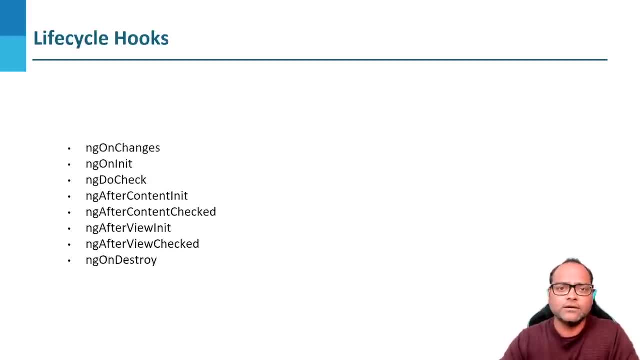 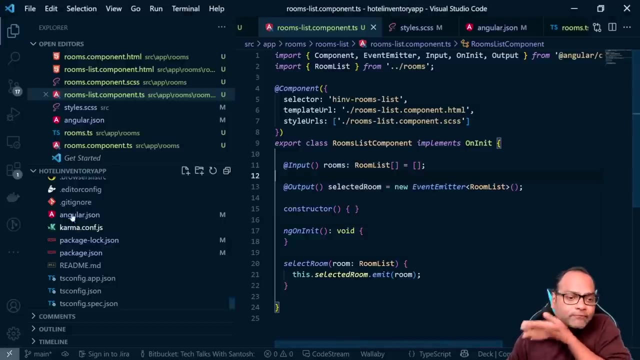 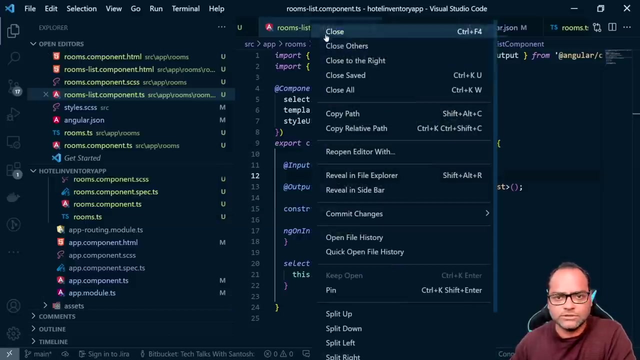 to change detection. So let's go ahead and go in depth and talk about how change detection works in Android. So let's go ahead and do that. So if you see our app right now, what we have is we have a child component, which is- let me just close this- We have a parent component called 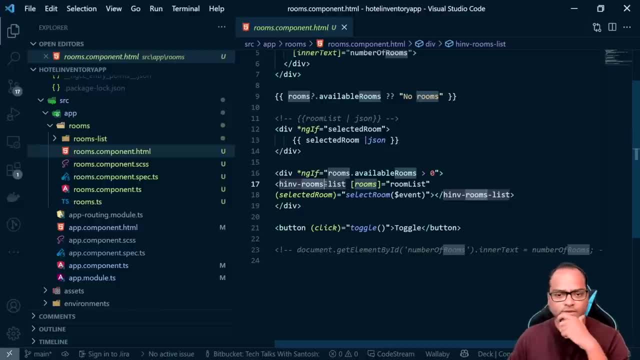 rooms component, and then we have a child component called rooms list, And then we have a top root level parent component And then we have a parent component which is app component. Whenever we do some action, the data needs to be updated right And the data or view needs to be updated if we talk. 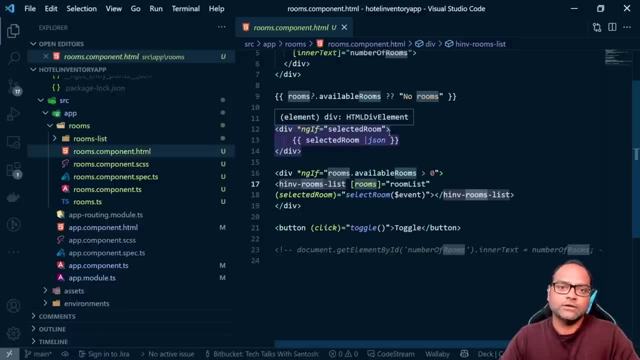 about, not the data- How that happens. So Angular does it via change detection, So it is actually internally handled by Angular. But there are multiple ways you can actually change change detection for your component. So let's go ahead and talk about change detection first. 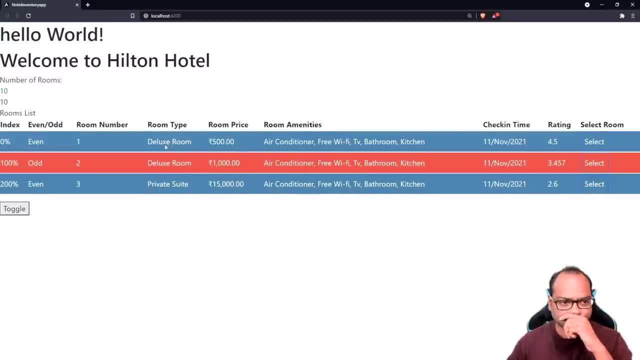 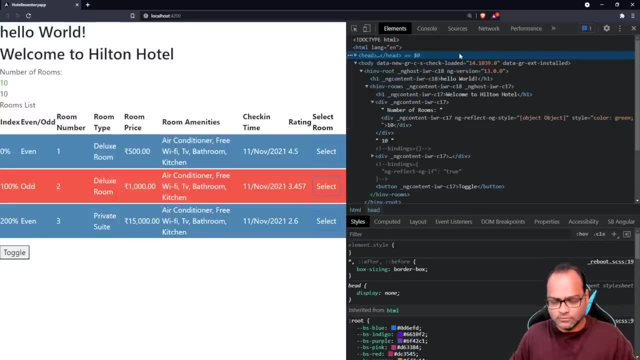 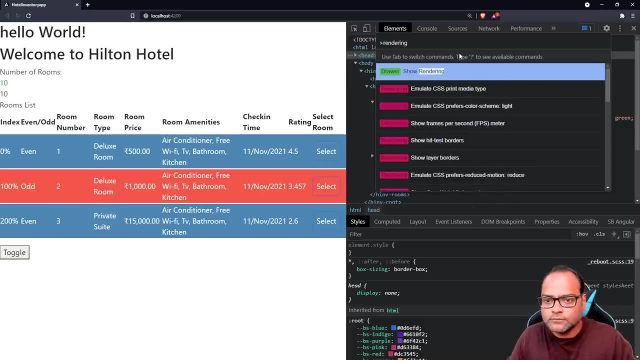 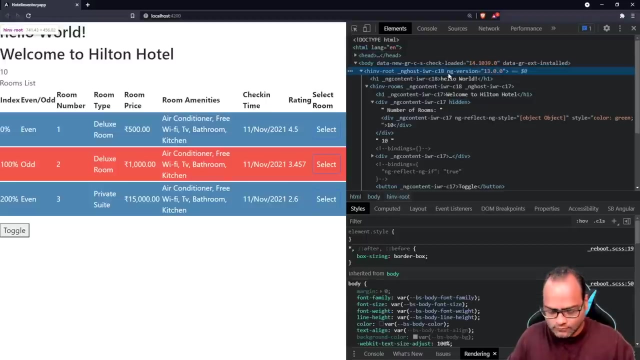 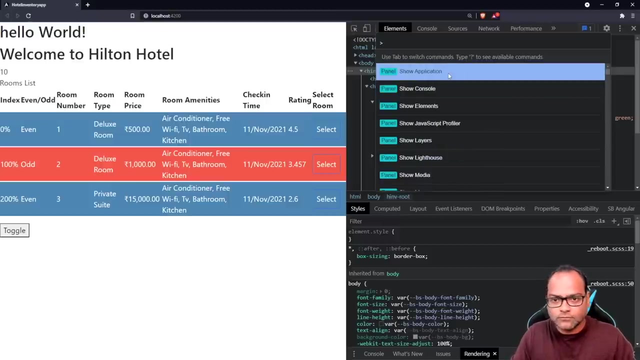 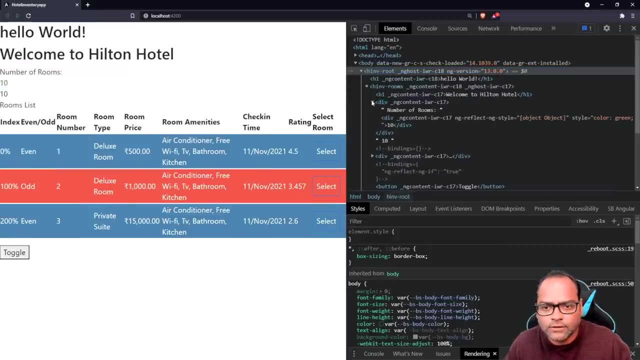 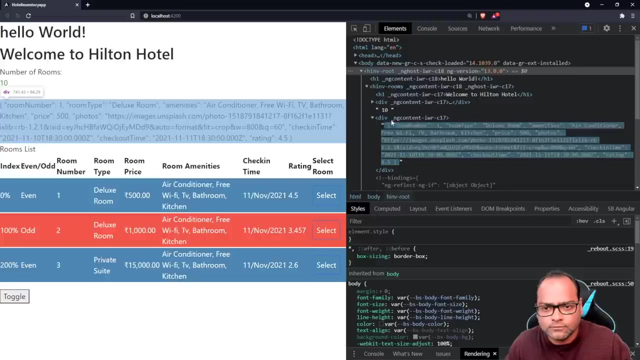 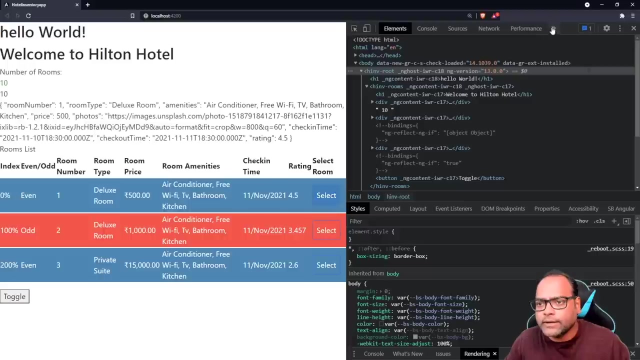 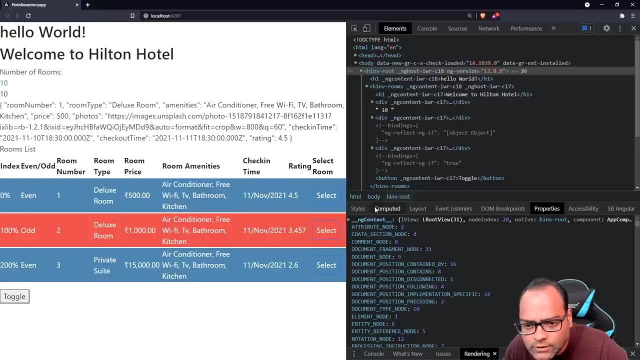 We'll go to the app. This is our app And I'm going to enable. So that's our app And I'm going to enable. It's climbing on. okay, now let's see, And we can go to panels. so we have styled computed layout rendering on. let me just 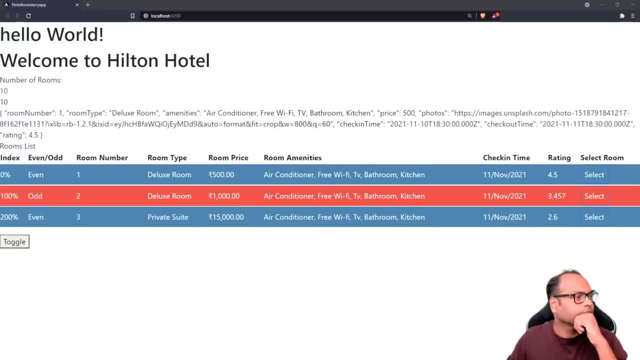 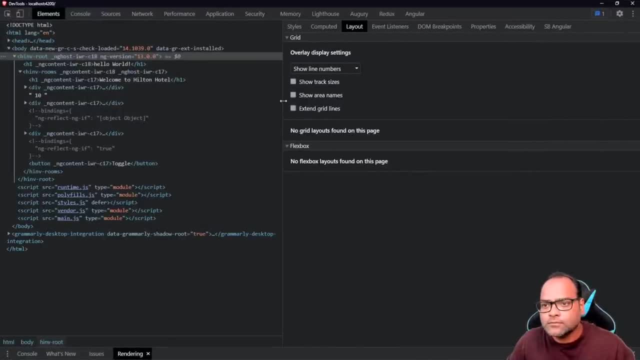 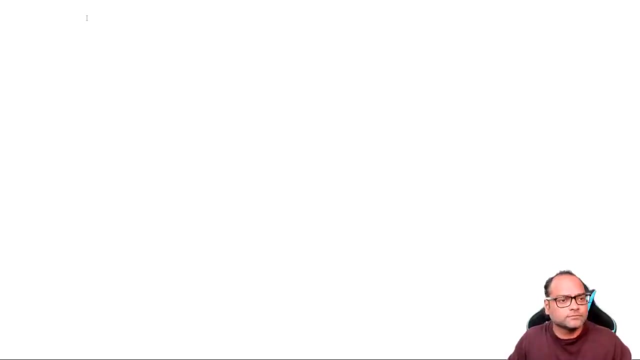 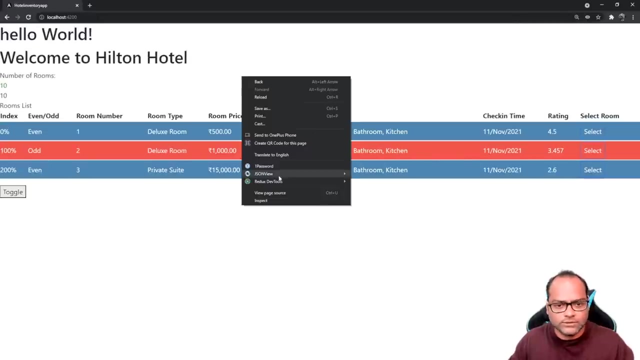 open it in another tab And let's see what we have here And show. rendering should be here. don't make points. no, computed layout should be missed. Okay, let's open this in Chrome. Let's open DevTools So you can press F12.. 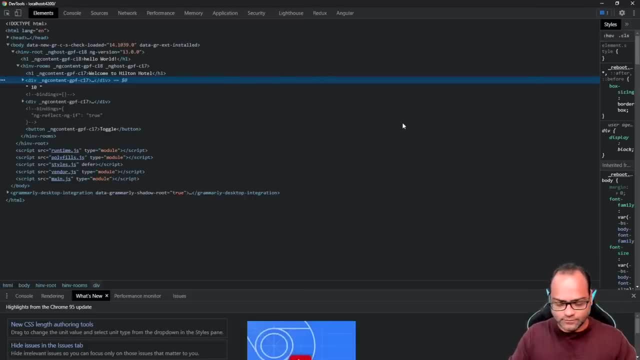 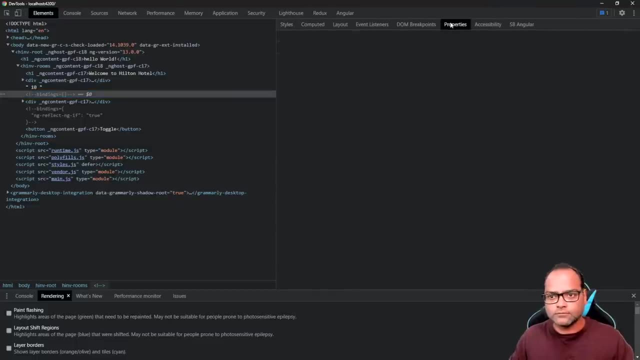 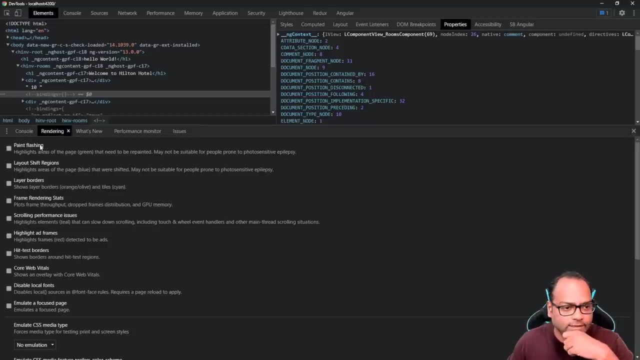 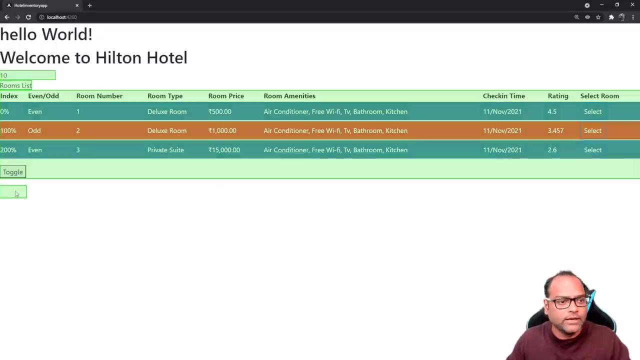 Or just right click and say inspect. Okay, so this is what I was looking at. So there is a tab called rendering which you can see, And let's click on paint flashing. This is the property which we I was looking at, and let's click here. 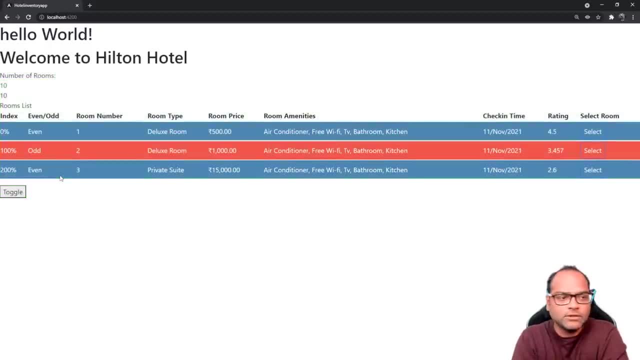 So some green borders. You can see right now What is this green borders? So this green borders are actually saying: these are the DOM elements which are getting changed. Are we changing everything? The answer is no, we are not changing everything, But still, whenever you click on some or you perform some action, Angular detect there. 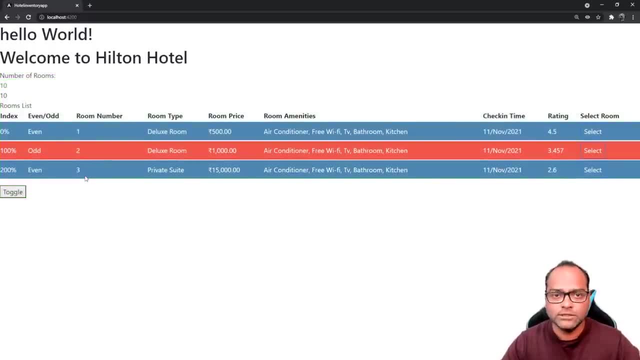 are some changes on your view and your view needs to be updated. This is by default, which happens inside Angular, But there's components which doesn't need to be changed. For example, this table right: Did we add it Or did we change it? 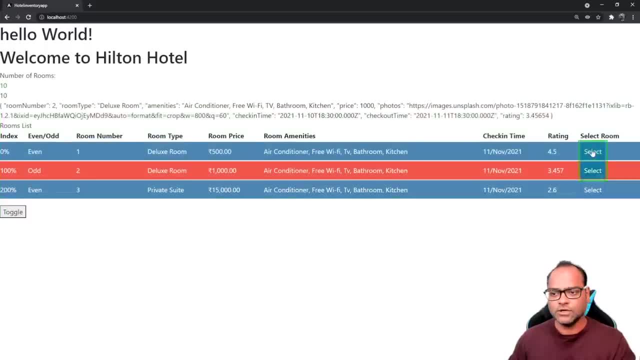 Or removed anything here. The answer is no, we did not, So this table should not change Why it is getting changed, even if I click on a toggle which is outside of like, this is something which is available on our parent component, if I'm not wrong. 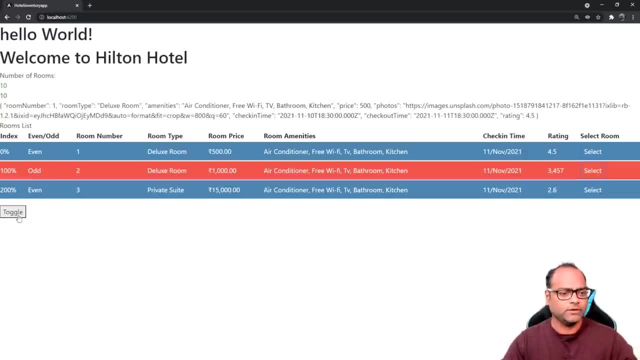 This is sorry. this is on rooms component, So this is on the rooms component, and then it is also updating the rooms list component. How is that possible? I mean, I'm not changing anything, but it is getting updated. So let's consider, like right now we just have two components. 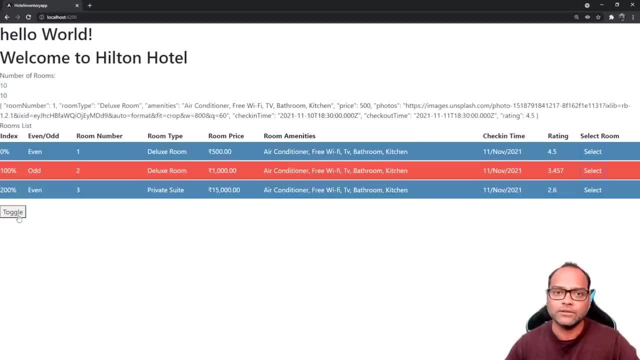 What in case? you have a lot of components on your view. what will happen? So change detection will run for each and every component. Can we avoid that? The answer is yes, we can. So let's see how we can actually optimize this change detection strategy, which is default. 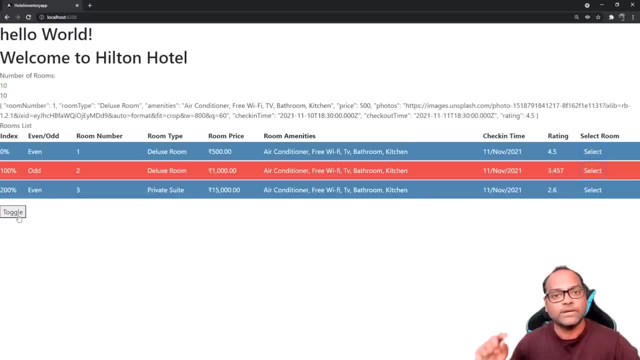 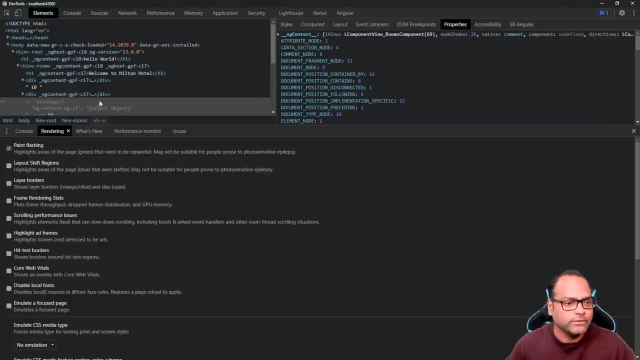 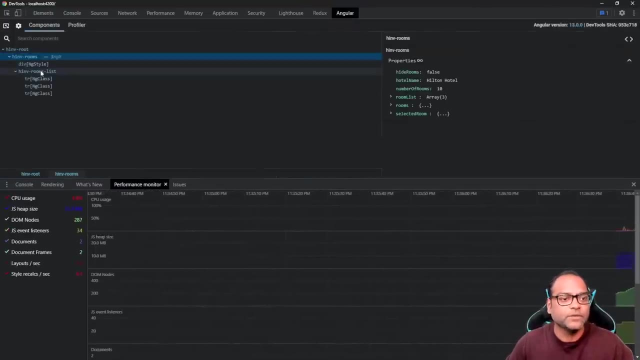 to change. detect changes for each component. Remember the way it runs is- let me just go back to depth tools And I'll go to elements here- And there is an Angular dev tools also, which is available now. You can actually see it here. 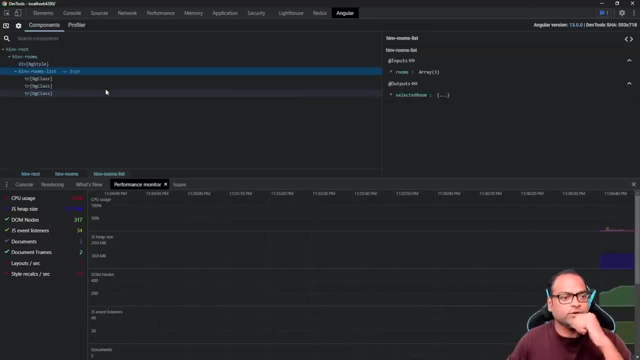 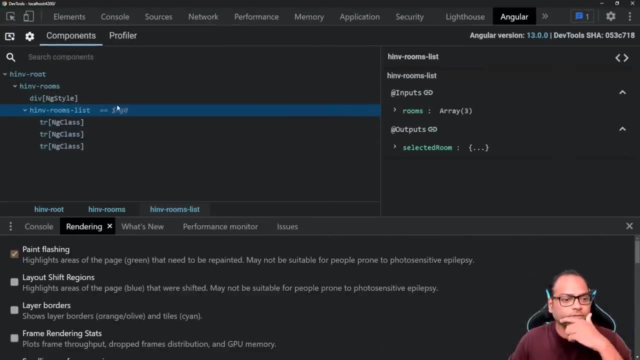 So let's say, down on tree, So this is your tree structure right now. Let me just zoom in. So this is our tree structure right now. So we have root, then we have rooms and rooms list. So in case someone performs action here, it it will of course send an event to the pattern. 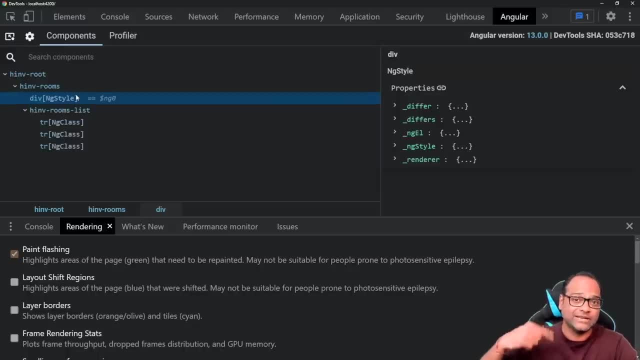 And parent will start running change detection for each and every component. So let's say I have rooms and then I have, let's say, employee, or let's say there is a. there is another view, which is to add rooms type. So what will happen is the change detection will run for both, even though I'm changing. 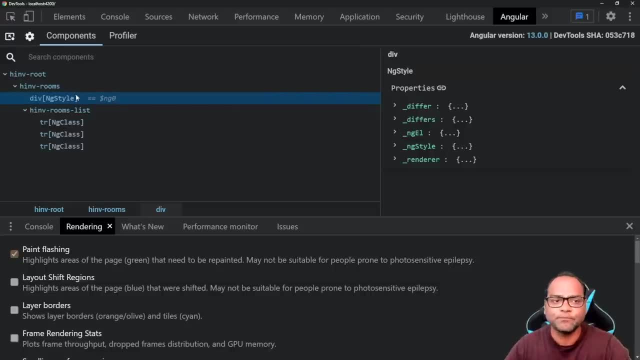 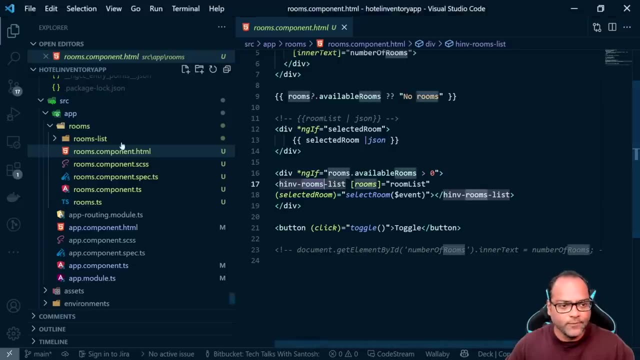 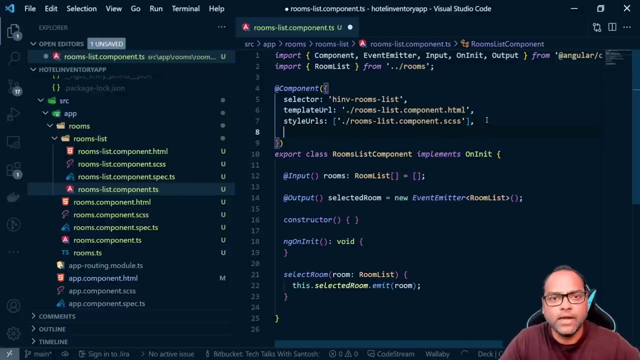 only rooms, or I'm changing something in rooms. By using change detection strategy, you can actually optimize this behavior. Let's go ahead and see that. So first, I mean, there are some rules before you can actually go ahead and apply change detection strategy to your component. 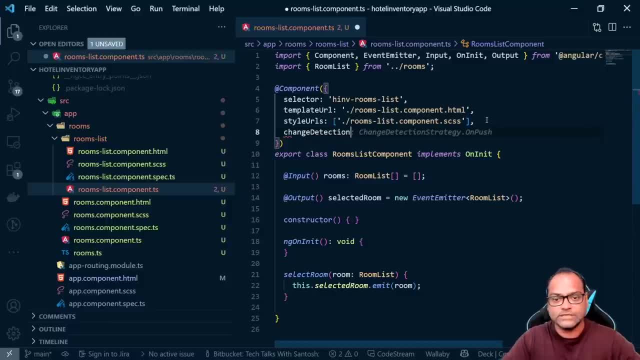 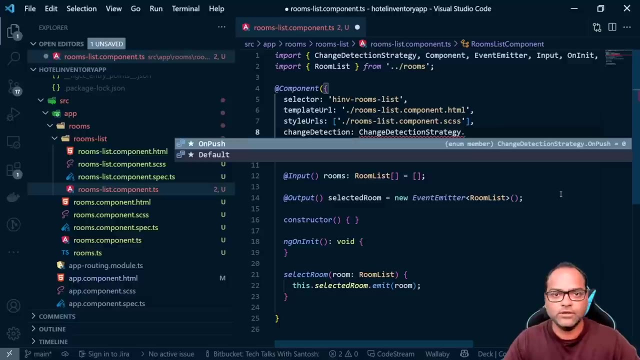 So here you can say: change detection, this is the property And there are two modes. by default it's on its default. Let me just import change detection strategy first, So we will get this intelligence. So you have default, Which is default when you, when we don't change anything. 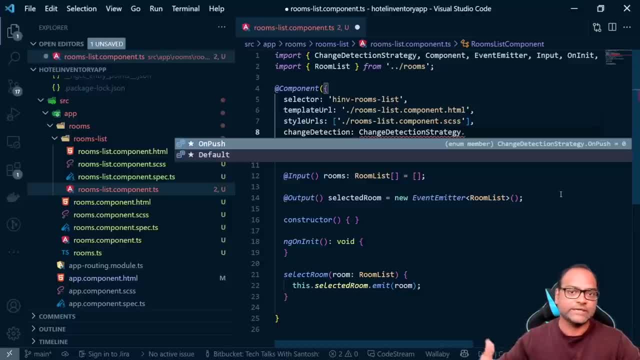 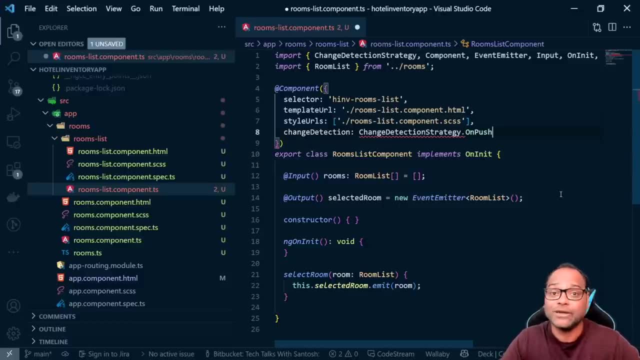 So any event will cause the entire change detection to run for your application. And then there is on push. before you go ahead and use on push, there are some requirements which you have to make, which you have to meet. On push, change detection strategy can be only applied in case I am not modifying some data. 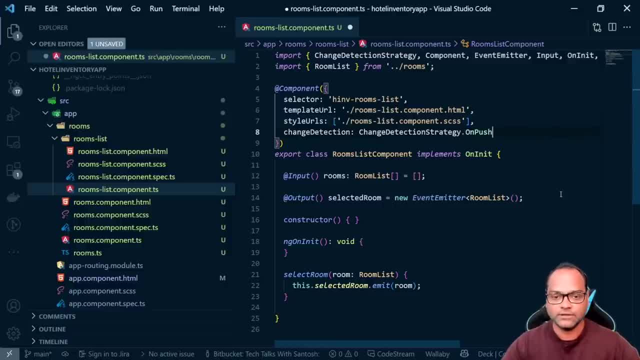 internally in this component how you can achieve it By using input and output. In future, you can also apply the same strategy in case you use some state management technique, For example, if you're using NGRX or if you're using any other state management library. 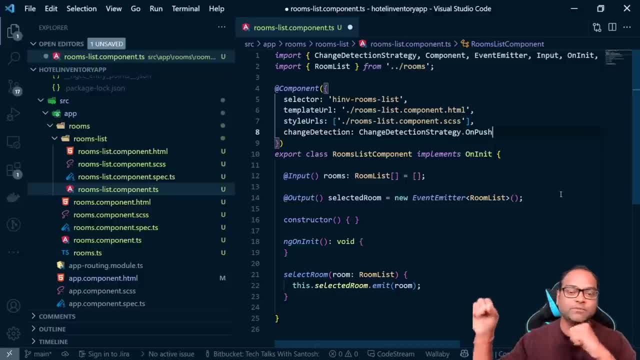 in that case also, you can move it to on push. Right now the state management part is out of scope of this particular course. So here we are going to apply it on rooms list component, because it uses input and output, So it doesn't rely. 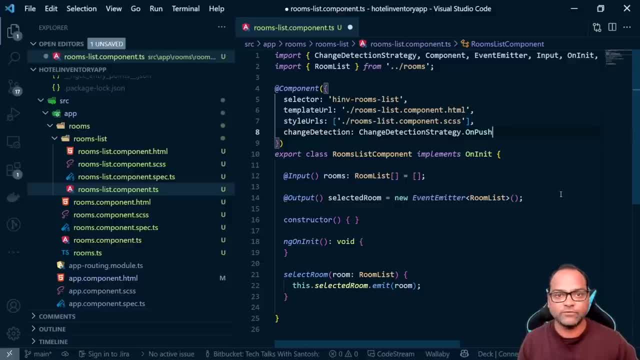 Or it doesn't change the data internally. it relies the data which is coming from outside, So it always knows that, if in case, the data is getting changed. So here let's move on to on push and to now to actually show you the difference. 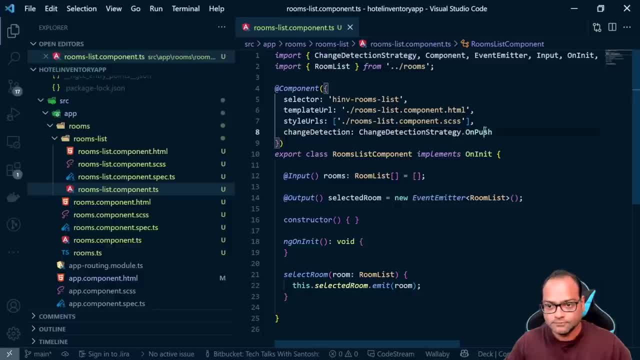 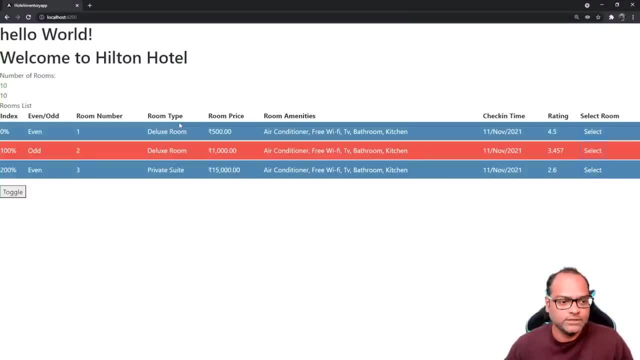 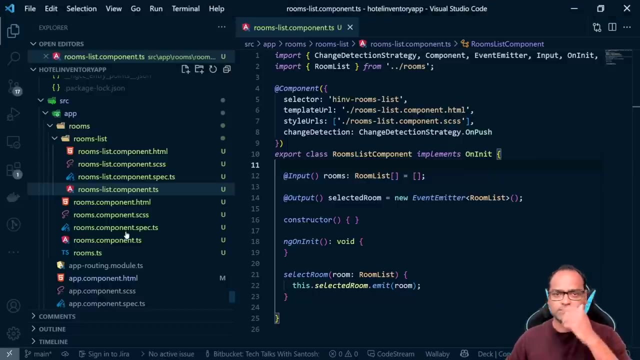 We have to do one more thing. Let's see that. So what we will do is we will write some small code To add a new record or to add a new room number. let's go ahead and do that. Just a small button. 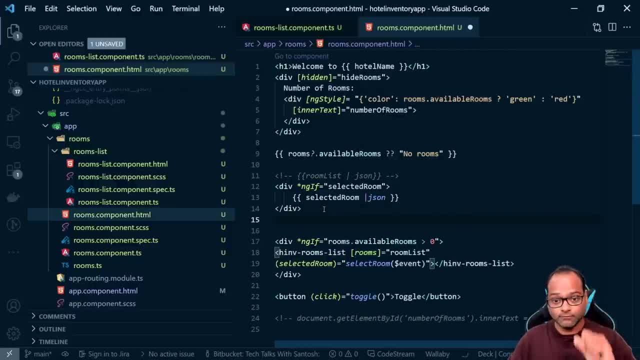 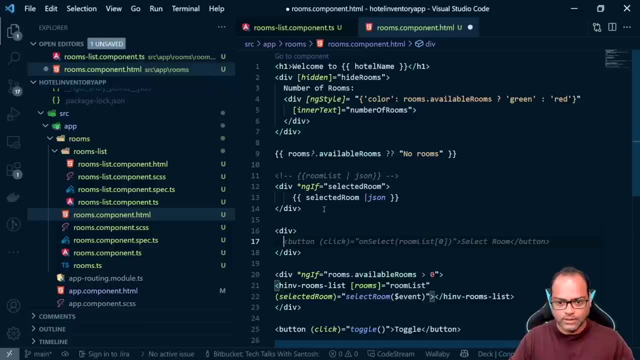 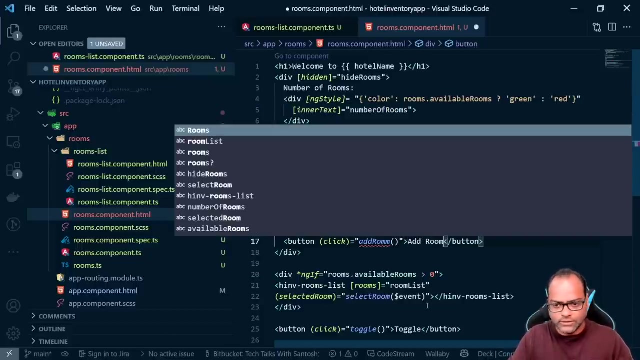 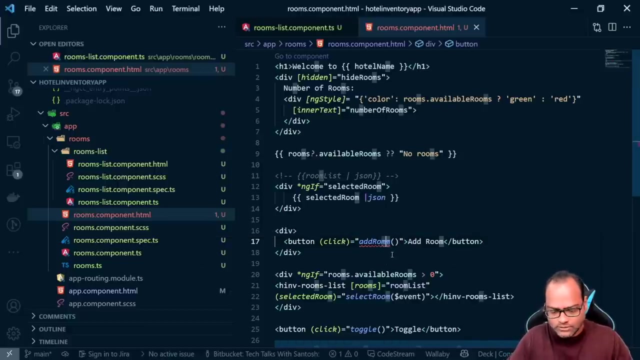 So let's do it here. So this is div And then we have button and I'll call it as add room And we will right now pass the static data. So I'll say: this is add room, Let's go ahead and again spelling mistake and let's go back to TS. 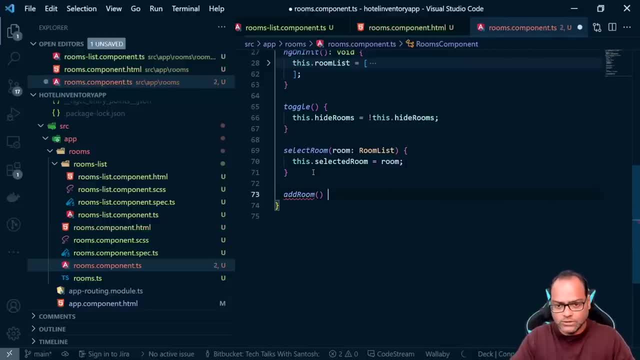 And here we will add a new room. So we'll create a room first. So I'll say: const room, which is type of room list, is equals to, And then we'll say: let's see what is the properties. room number four: 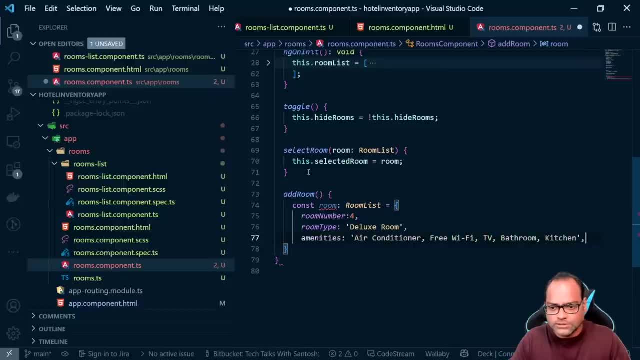 And then there are room type, there is amenities, there is price, there is photo, So we'll just copy the one from the existing property- And there's checking time and then you have checker time and then you have rating. Okay, So this is our new room data, which is available. 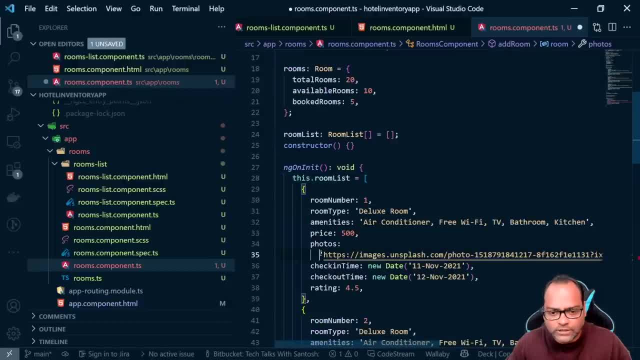 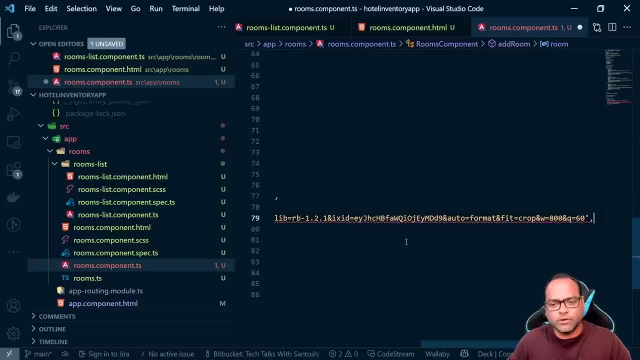 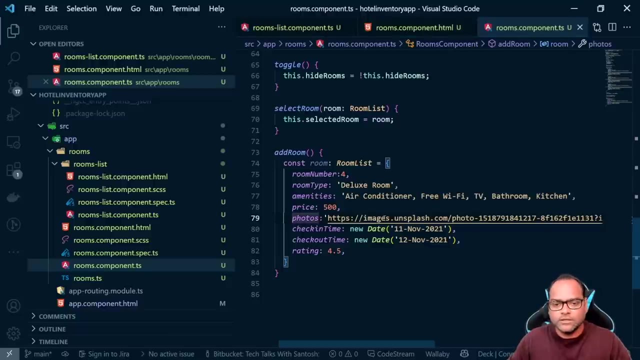 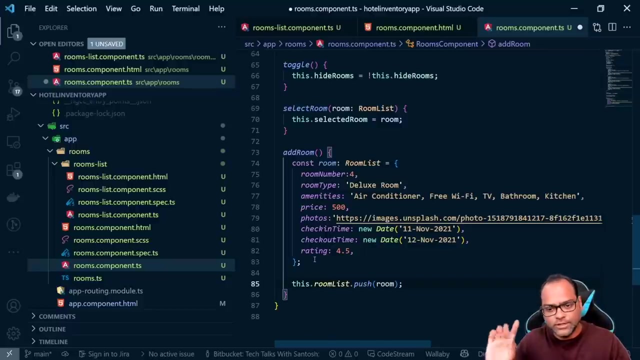 Let's copy. Let's copy the photos: property here, Because all the properties are required as of now. We have to pass each and every property And after this I'll say this: dot, room, list, dot push. So let me just do this room list dot push and let's go back here and comment this out. 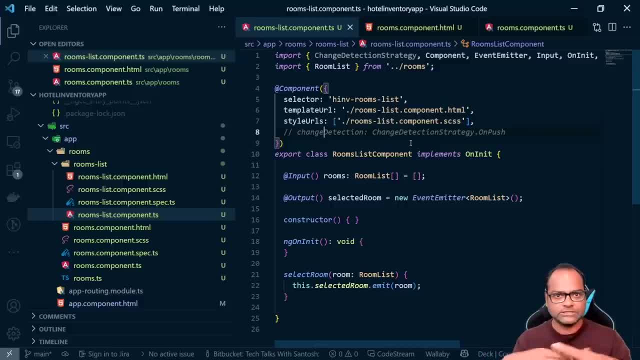 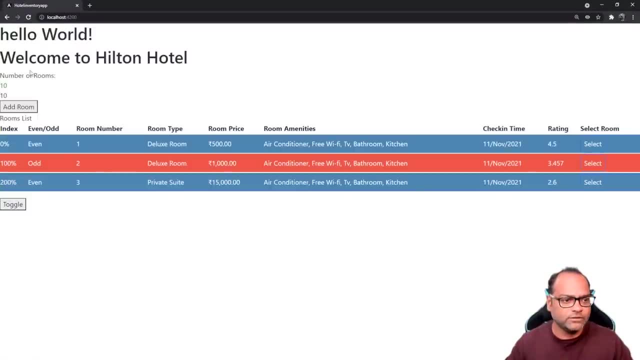 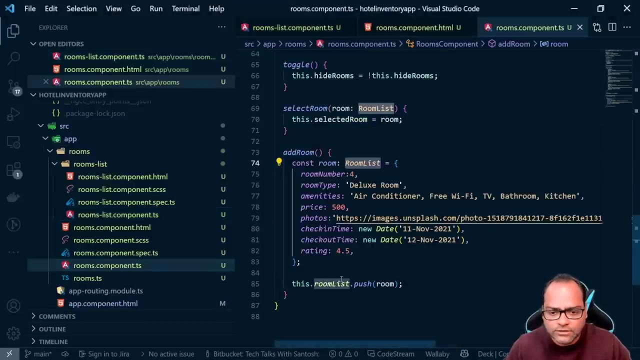 So we are saying right now: my change detection strategy is default, So it means any action is performed. Just go ahead and run the change detection for everyone. Let's click on add room- see room list, room list dot. push and then you have room list. 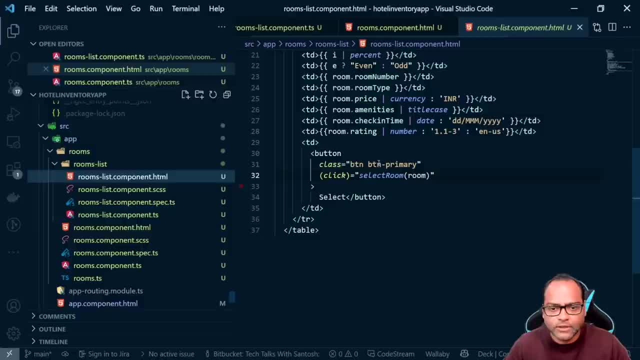 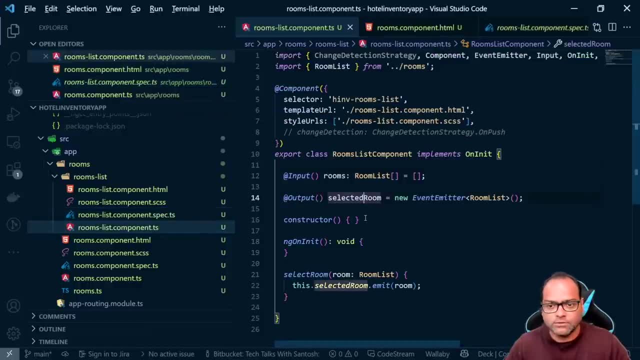 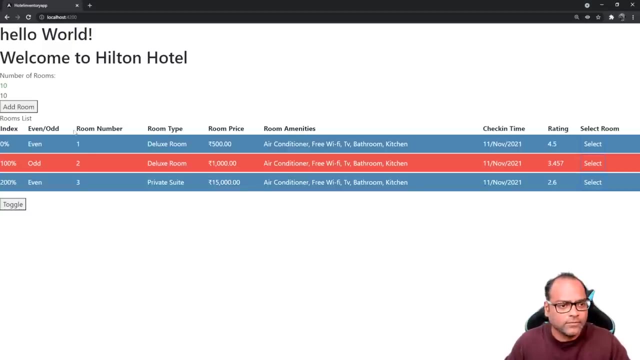 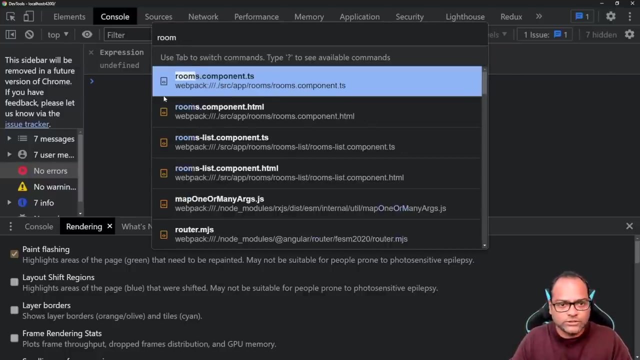 available here, So should work. Let's see. Okay, Okay, Okay, Okay. Let me just save this file again, because probably this is happening because it is not able to identify the change detection strategy. Let's see if there is any error. let's go to oms: component dot ds. 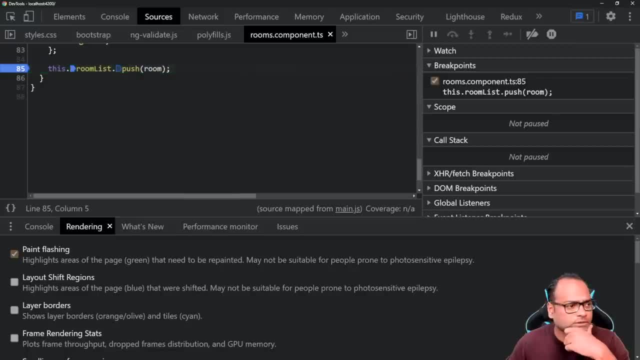 And what we have is this data. Let's go to oms component dot ds, dot rooms list. So rooms list we have. Okay, We already have the record available here. One, two, three, four is added twice, So it should work. 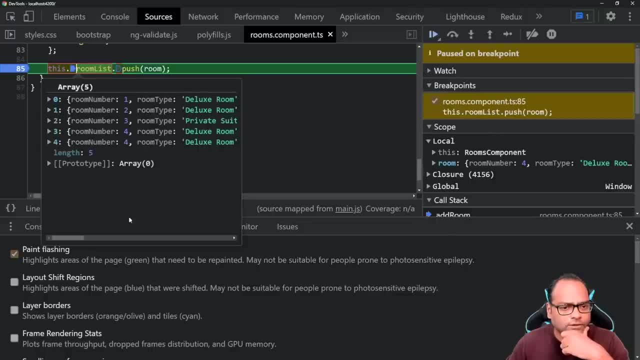 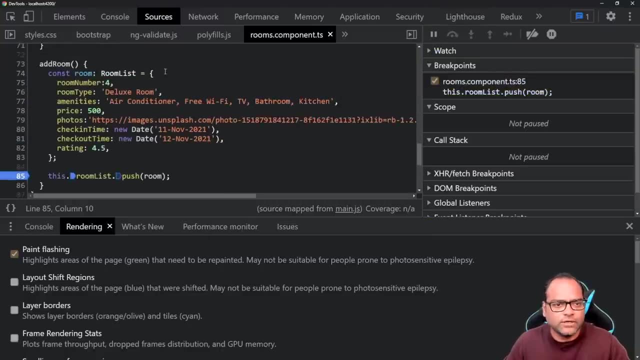 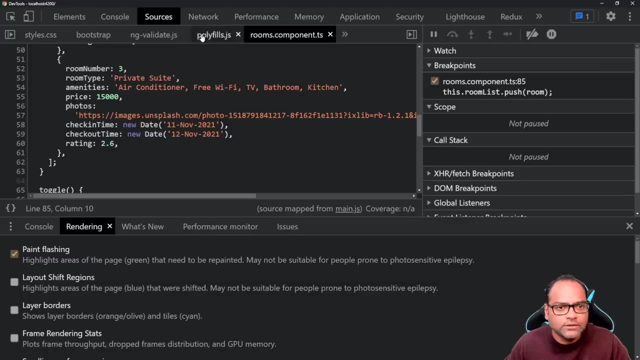 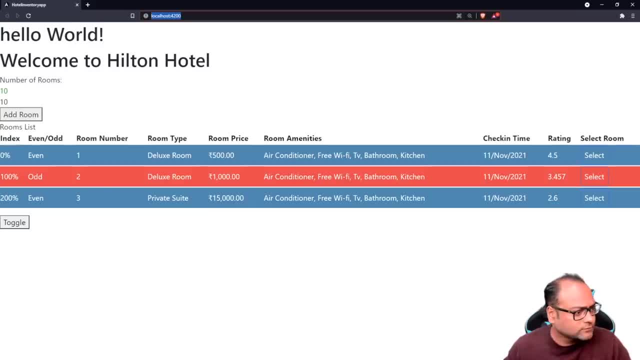 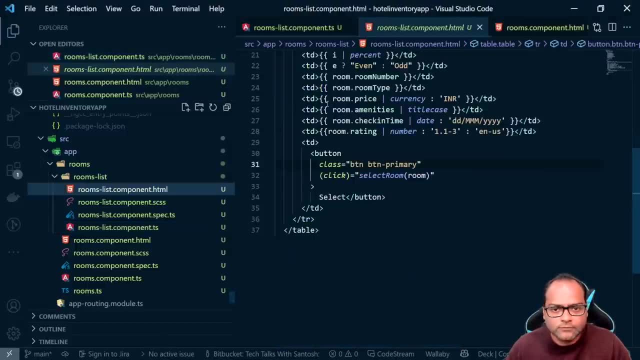 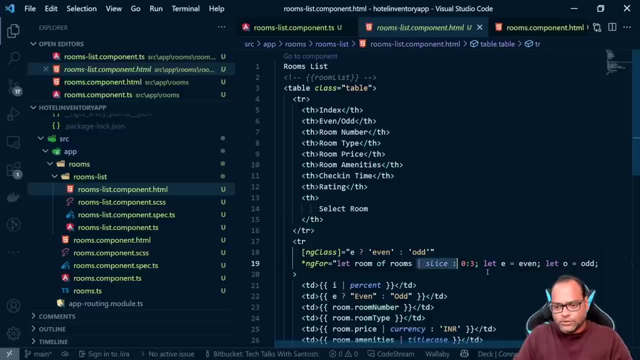 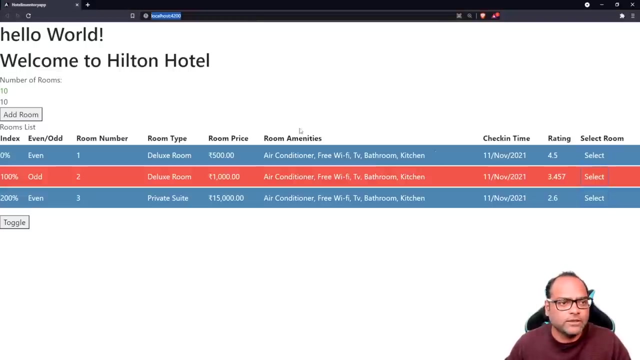 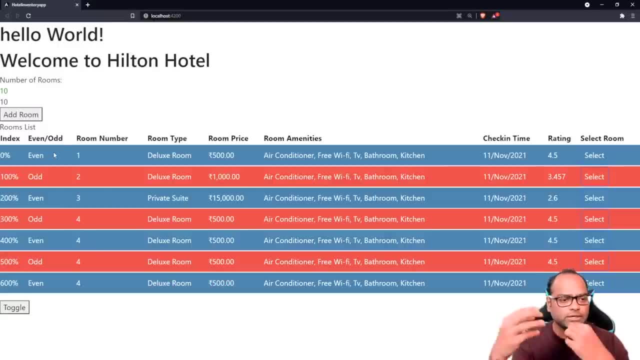 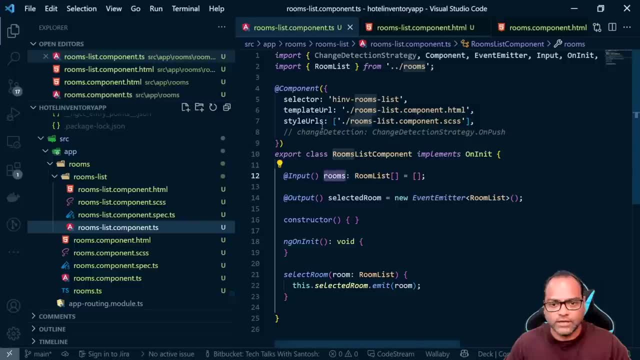 So you can see it is working fine and whenever you click on Add Room, the record is getting added. Now let's keep the record. Okay, change this code as as it is and let's go ahead and apply change detection here, because this is 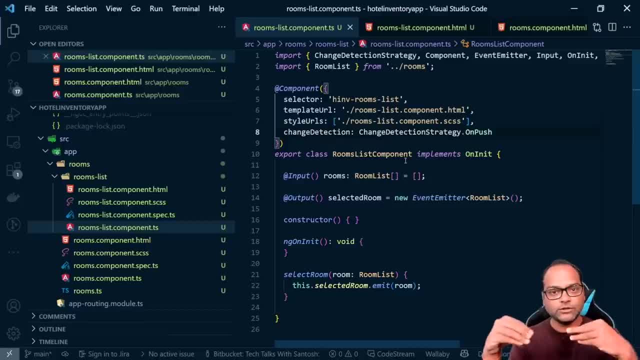 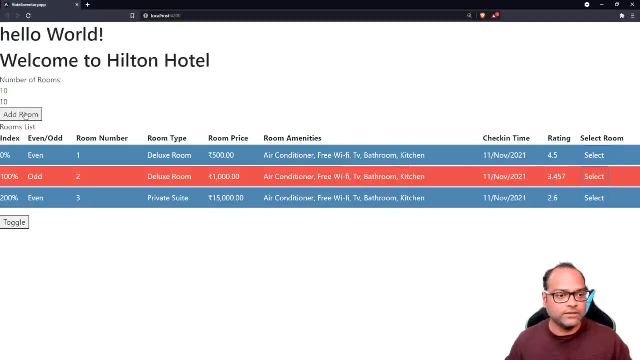 really important. i mean, uh, you, uh. you might have understood now that, okay, why to use on push in strategy? because we are not modifying some data here and the data is actually coming from outside. but there is one more important concept which we need to understand, so let's go ahead and see now. 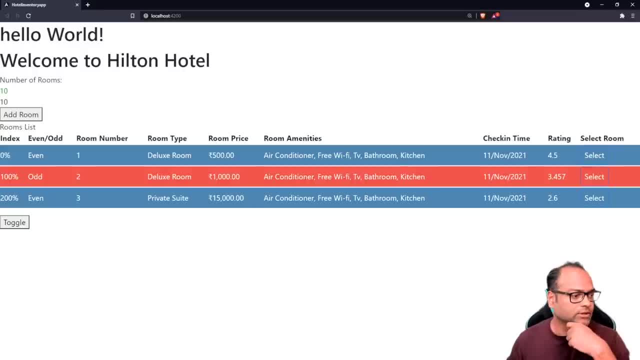 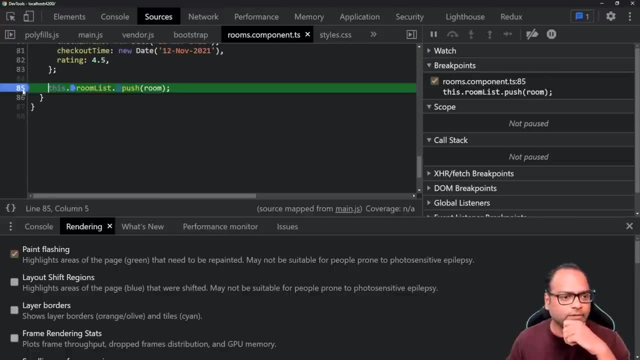 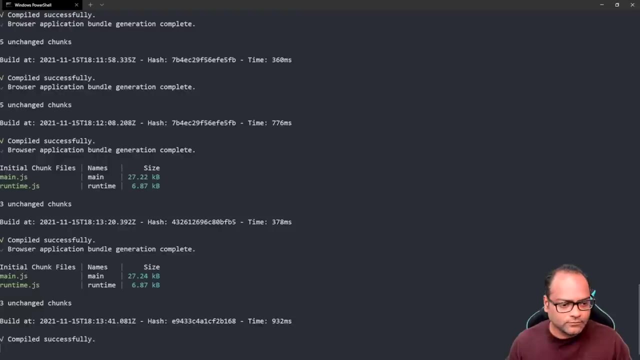 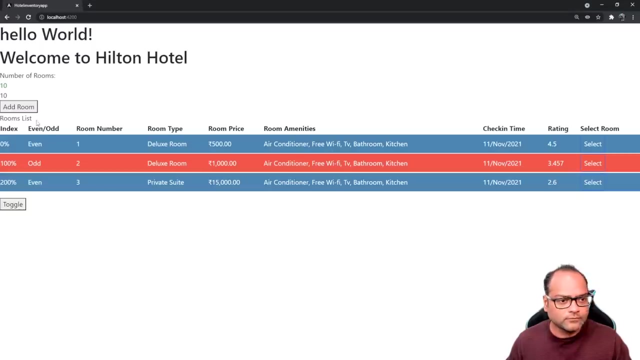 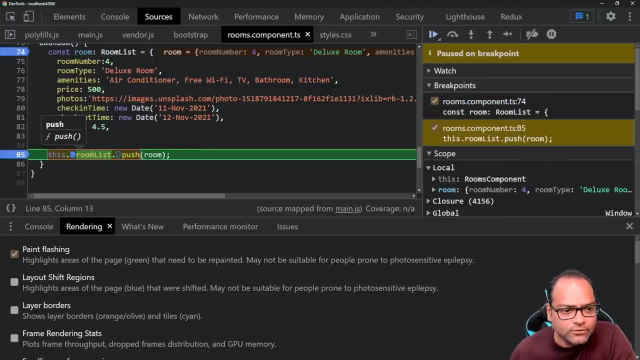 you can see, actually i'm clicking on add room and nothing is happening. but let's see a magic. so i'll go to, of course, devtools and let's click add a breakpoint here, click on add room. okay, so you, you can see you your room list right now here. 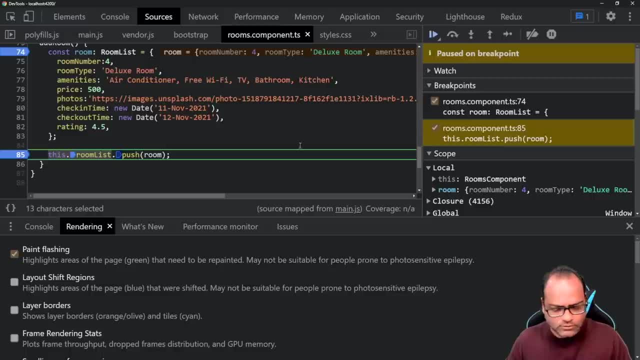 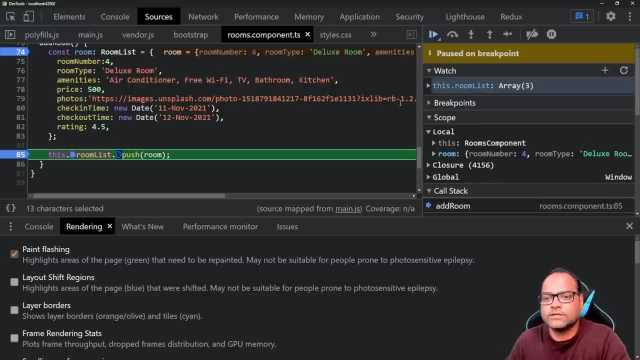 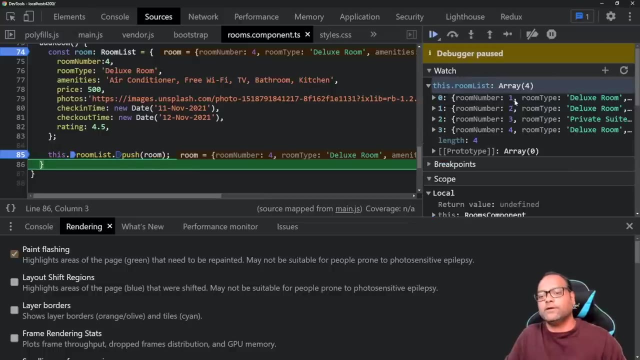 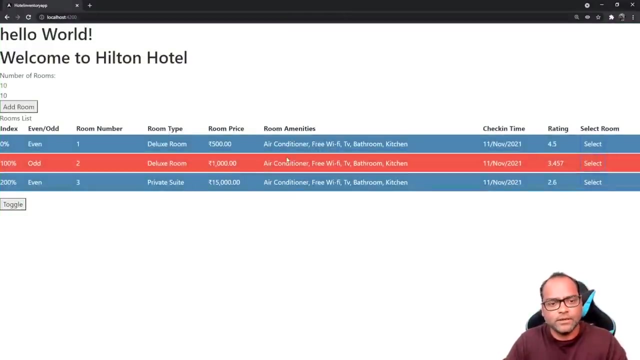 okay, somehow it is not able to show, click, add in the watch and let's see what is available here, so you can see. okay, your uh data has f10, four records here. so you have one, two, three, four and let's move on, but here you still have three records. why so? because now my component, which actually 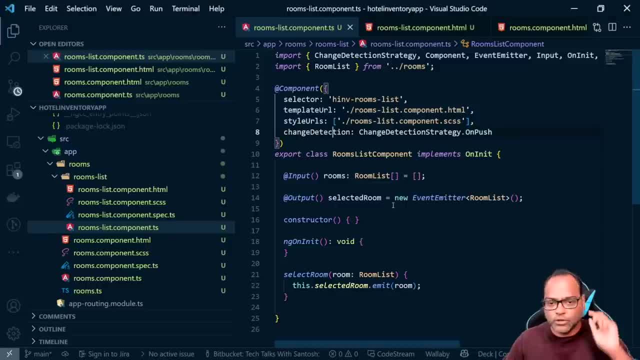 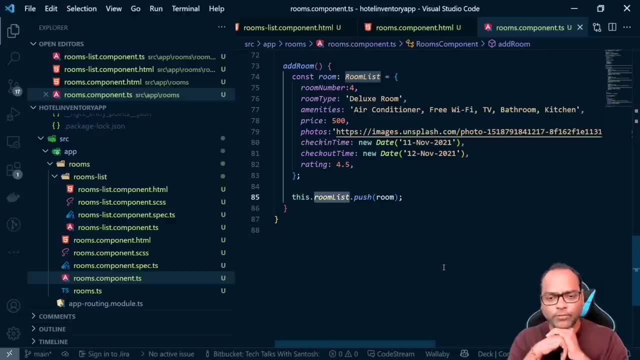 is on change detection strategy. on push, there is one more requirement which you have to, which we have to meet here. let's see what is happening here. so this room list property which is getting binded to my child component, what we are doing right now, we are actually pushing and record into this particular array. 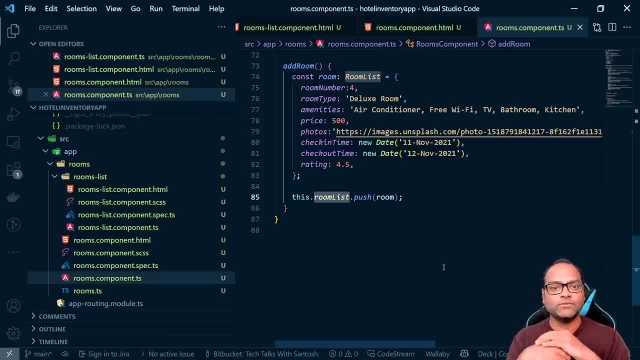 so this is where you have to understand the concept of immutability whenever you are working with change section strategy. on push, the data which you are trying to assign should not be mutable. so it means when we apply a dot push, what happens? we actually change the room list property. the concept of immutability says we should always return a new. 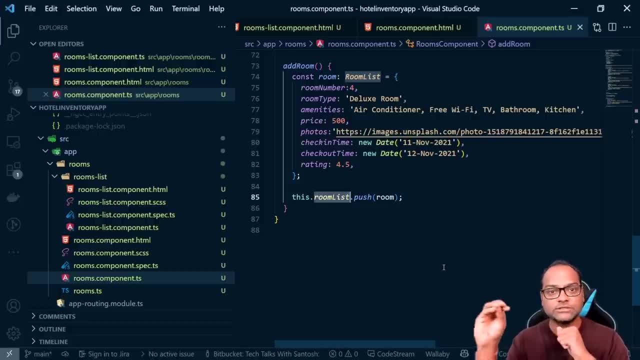 instance. remember this because it is really important, because in future if you try to use some state management technique and try to do the same stuff, you have to understand the concept of immutability, because entire state management thing works with immutability. so here we are saying, rather than actually modifying, 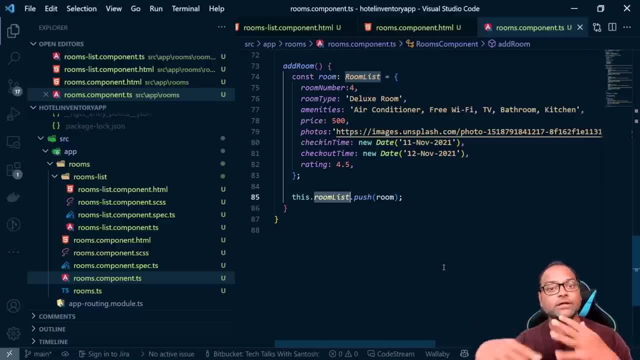 room list directly. what we need to do is we have to return a new object every time we modify this instance. it can be an object, it can be an array, whatever, but in case you are trying to modify it, return a new instance. how we can do that? so there are. i'll show you a syntax which is very useful. 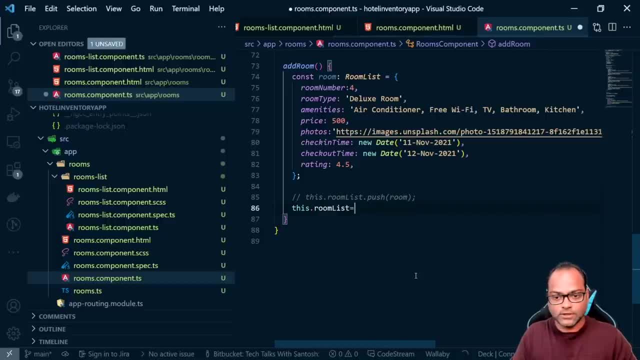 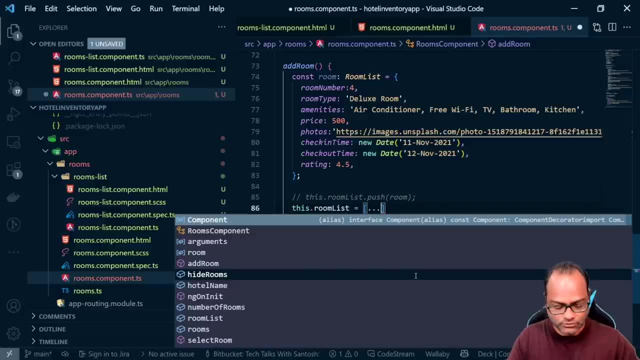 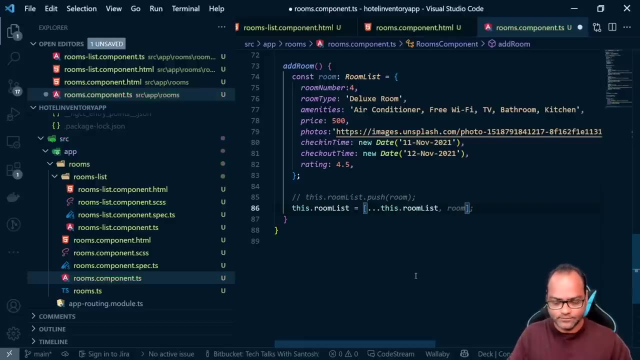 so you can say this dot room list now is equals to: i can say dot, dot, dot, three dots. it is called spread operator. so i'm saying this dot room list, which means keep the existing data and add the new record, okay. so this spread operator will say: okay, this in this array spread the previous data. so in case, 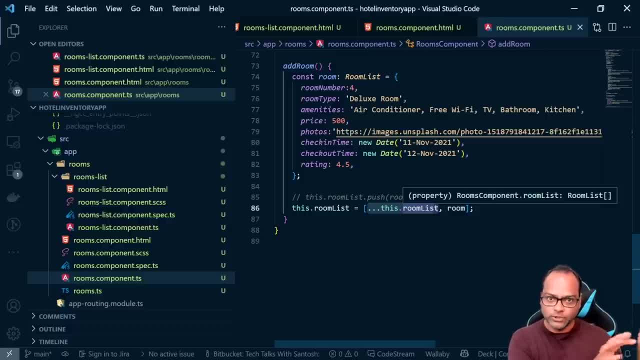 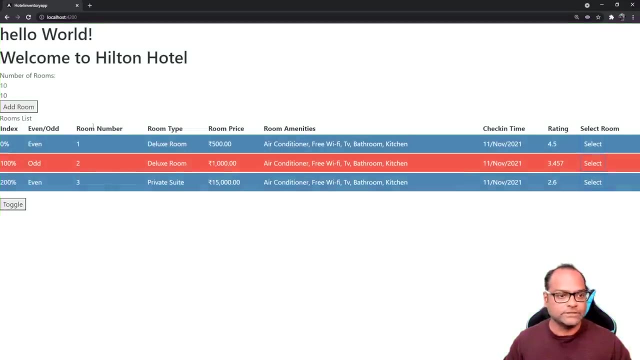 i have three records all present already, so three add three records plus the new record. click on it again. what will happen? so it will have four records and the next record will be added, which is fifth record. let's try to run this and see how it works. so let's click on add room. 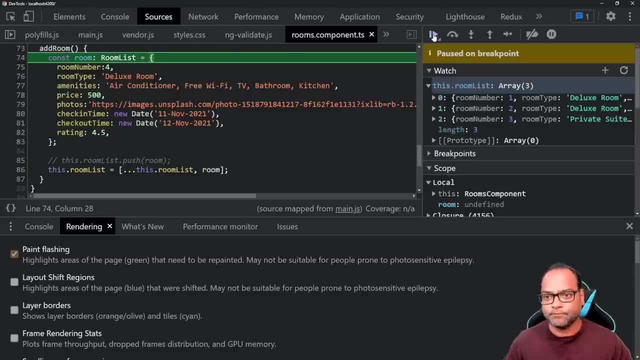 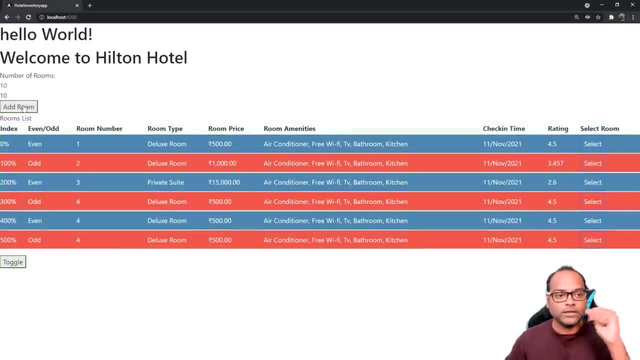 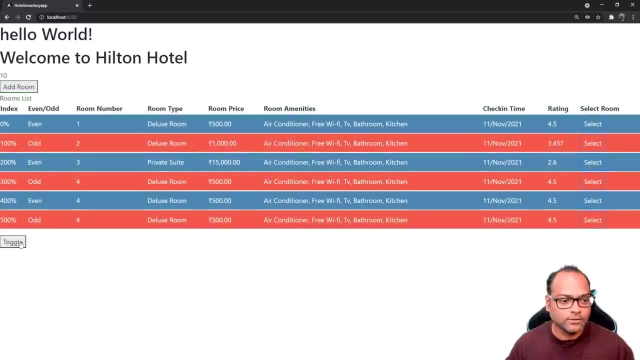 and um, of course, i will remove the breakpoints and you can see. now a new record is available. click on add room: again, a new record is available. so now, uh, the advantage of using on push. let's click on toggle. so here what will happen is now, as my rooms list component is on change section, strategy on push. 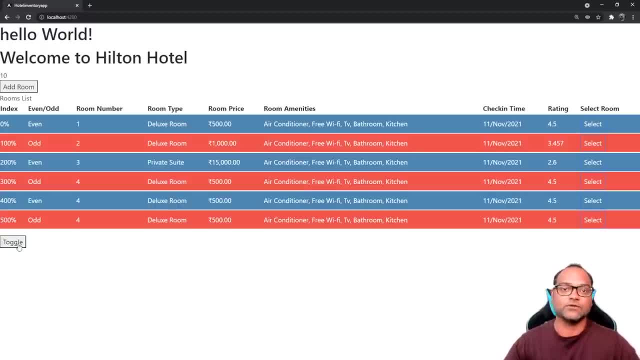 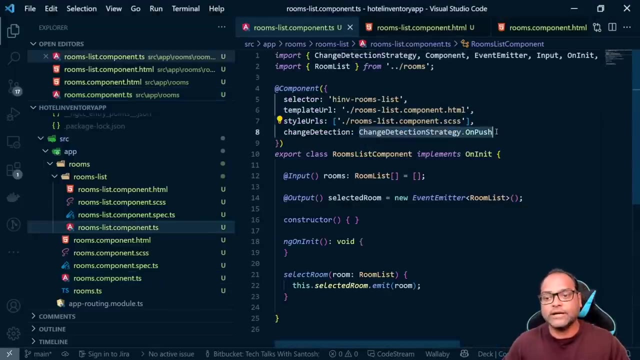 the component. also, sorry, the change section tree will check. okay, if this component is marked as on push, it means i have to only run the change direction in case something changes inside this component. so here this property will make sure that we are not running the change detection for this particular component until and unless needed. but 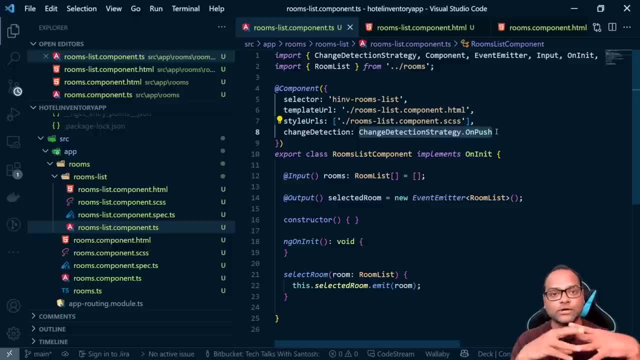 keep this requirement in your mind. first, of course, your component should not change the data internally. second, in case you are assigning or passing some data, it should be: uh, it should actually come from the parent component. right, it should or it should not. uh, it should the property. 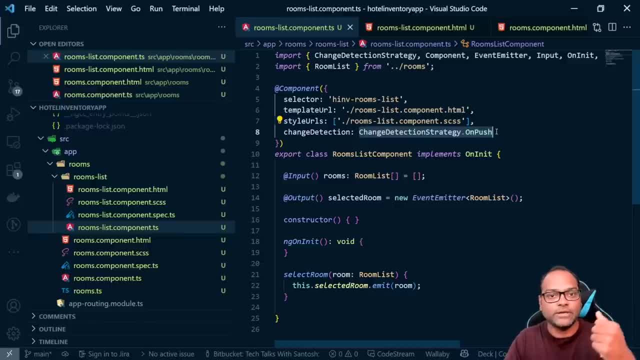 should be immutable. so it means, whenever i am assigning a new property or new value, it's the whatever your let's say, if you are using state management, state management or like ngrx or ngxs, they always return a new object. whenever i try to modify something, same same concept applies. 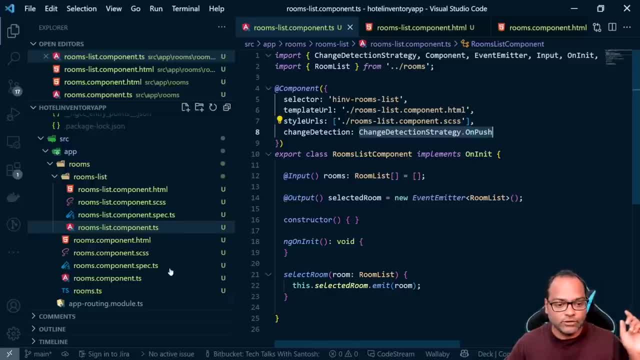 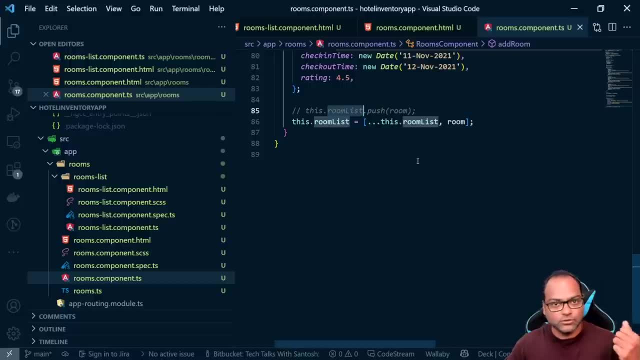 here. so in input property, what i did earlier was i tried to use dot push. what dot push did? it modified the room list property. so right, it actually mutated the existing object. but it should not do that. it should be immutable. so it should not do that. it should be immutable. so it should not do that. it should be immutable. so it should not do that. it should be immutable. 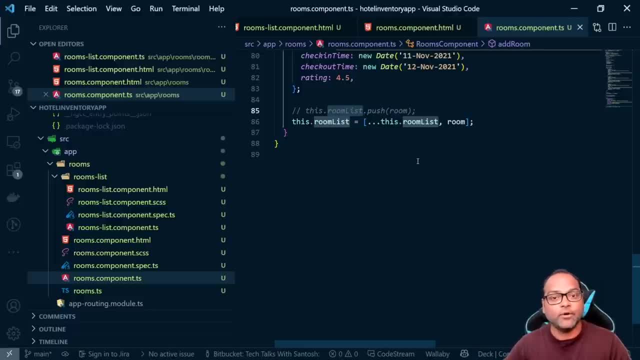 it means, whenever i am trying to apply some uh or pass some data to my child component- and i have changed section strategy on push- it means i have to apply a new instance or give pass a new instance every time. so what i did, what we did: we changed this code from this push method to this new uh. 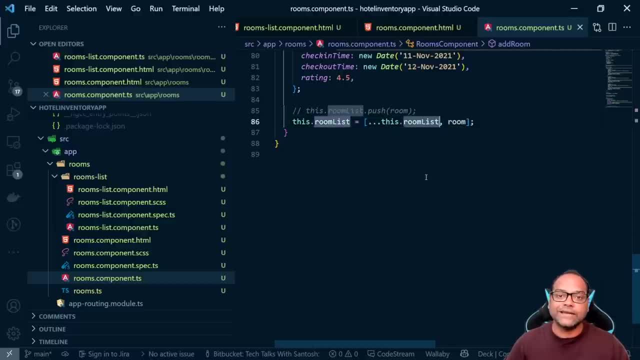 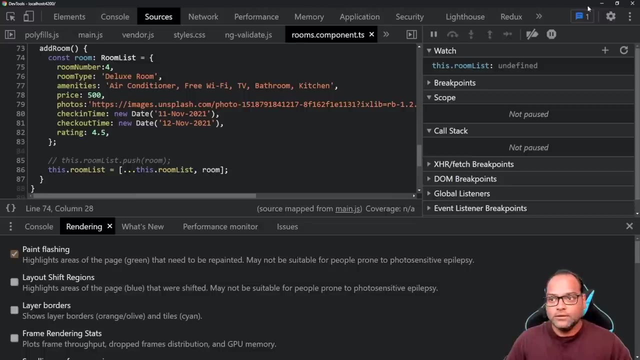 code where we are using spread operator to make sure: okay, the existing data is already available in array and the new record gets added. so this is related to change detection strategy on push. now go ahead, and let's go ahead and talk about ng on changes. so close this and 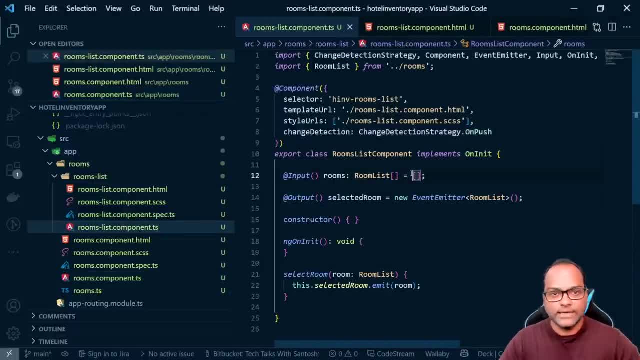 here. so on ng on changes property or ng on changes lifecycle look can be applied on a component which has input property. remember this: you cannot apply ng on changes lifecycle look anywhere else. you can only apply on component or a directive which has the input property right now. 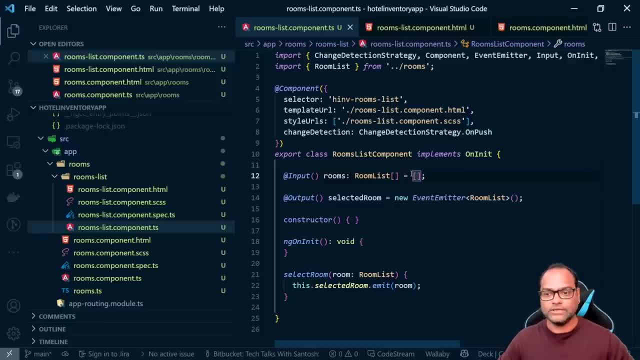 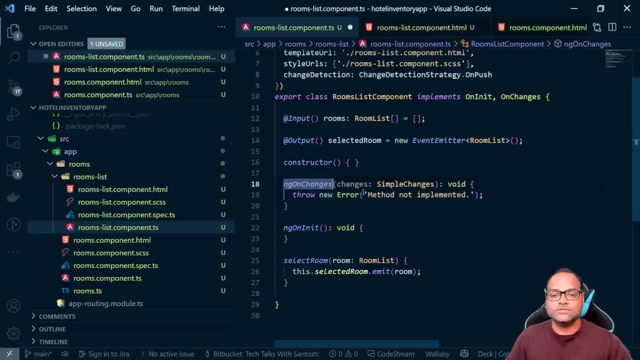 our component, uh rooms list component- has input property. so let's see how what it does and how it behaves. so i'm going to use in on changes and let's implement interface. so, uh, you can see engine changes, get some property which is changes of type, simple change. 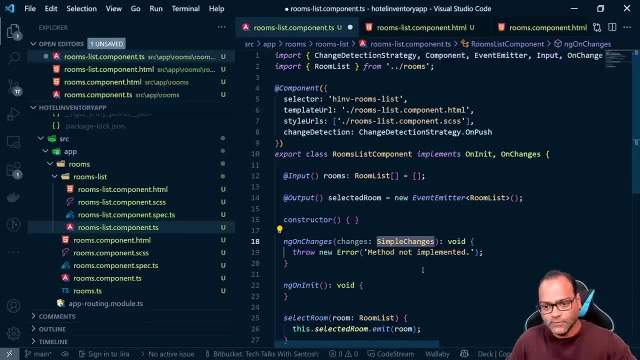 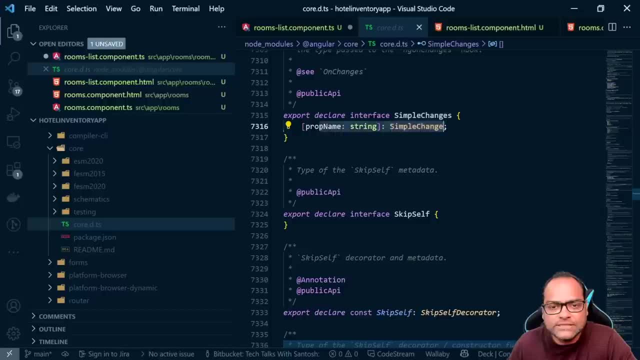 and let's see what simple change is. simple changes, sorry, simple change- is also an interface. so here you can see simple change. so what it has is it's a. it has a property name and some metadata. so let's see what this method is: simple change property, so it will give you. 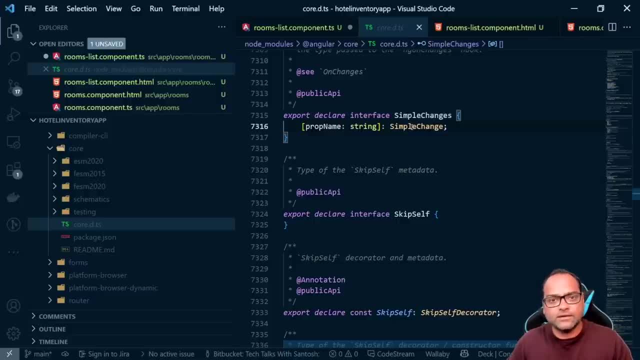 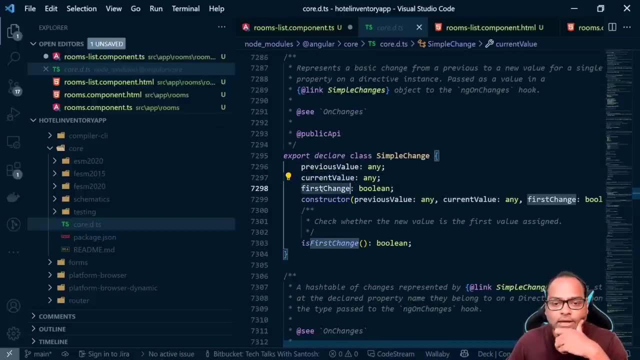 sorry, it will give you some information, like previous value, next value. so let's see here- so you have previous value, current value and whether it's a first change- and there is a is first change property as well, boolean property as well- what we can achieve using this. let's go ahead and do that. 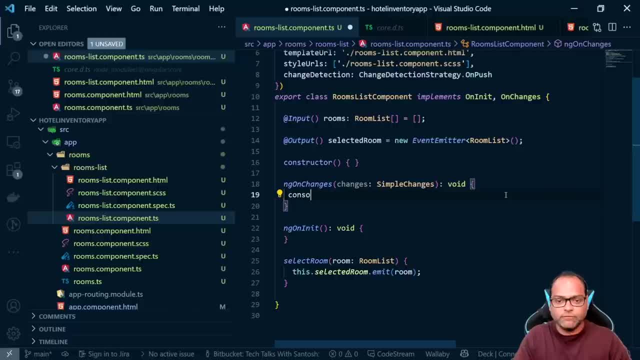 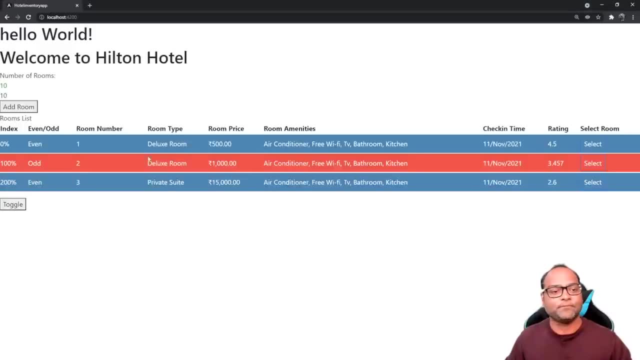 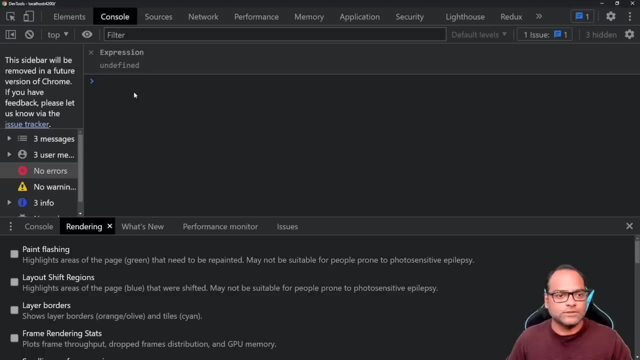 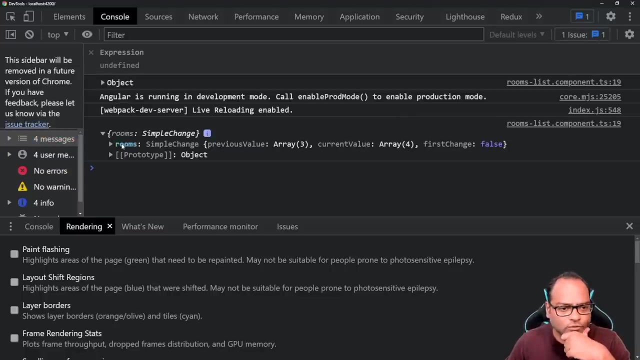 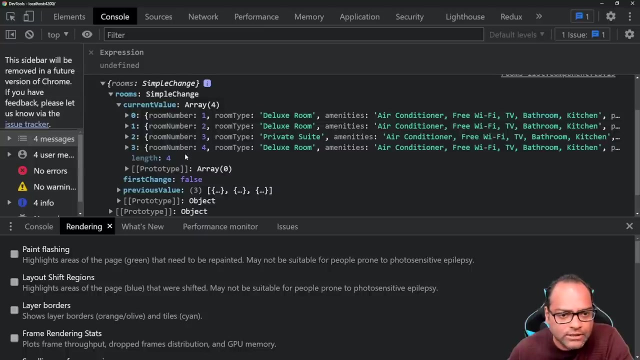 here right now. uh, what we will do is we'll just write consolelog to just figure out what's happening here. so what actually ng on changes does, let's inspect, let's go to console. so let's go to console and click on add room and see here, so you have some data which says rooms, simple change. current value is like this: 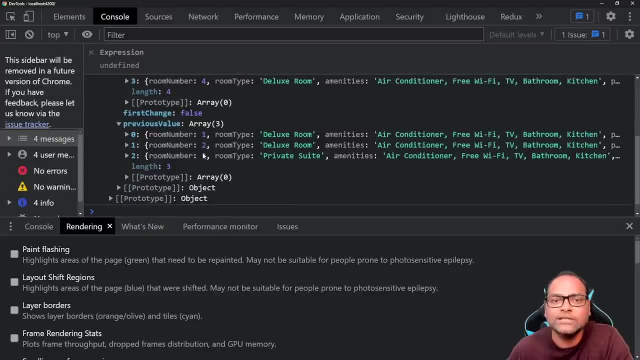 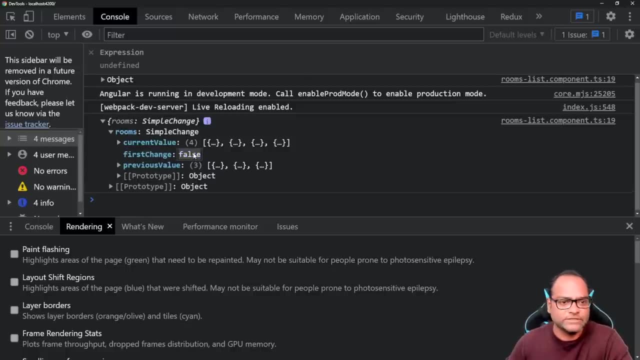 one, two, three, four, four records. previous value was: one, two, three, three records. is it a first change? you can also find that property. so it says first change is first change property. so first change is false. it means no, it is not a first change. it is because previously you can see there was one. 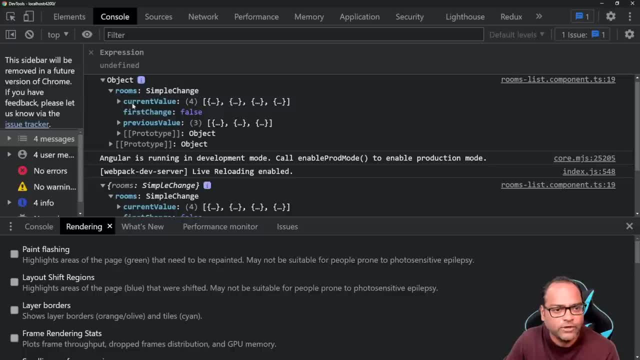 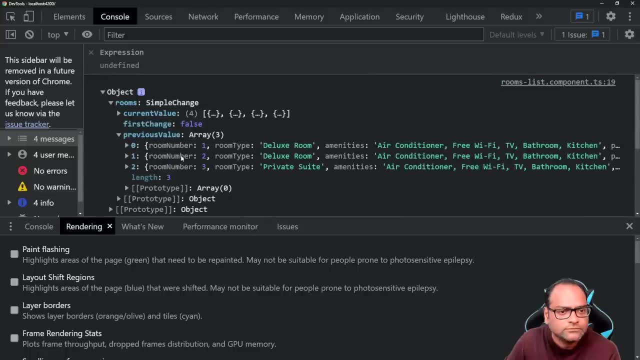 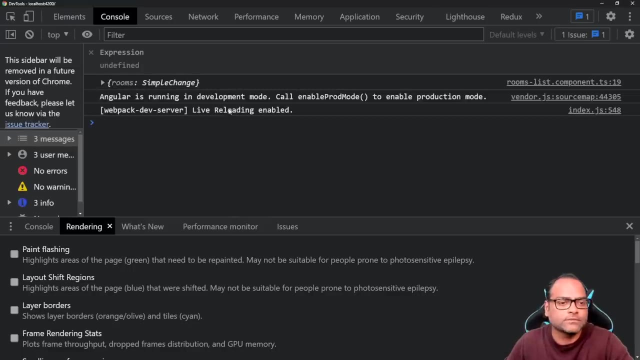 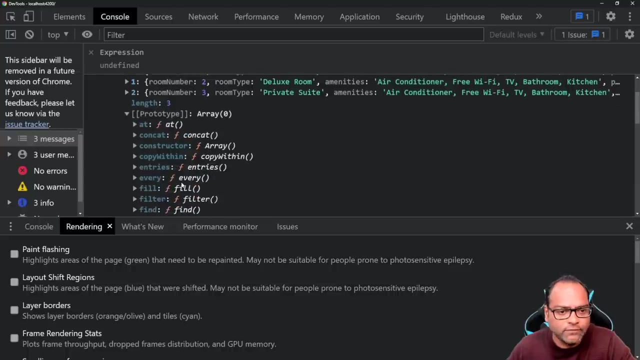 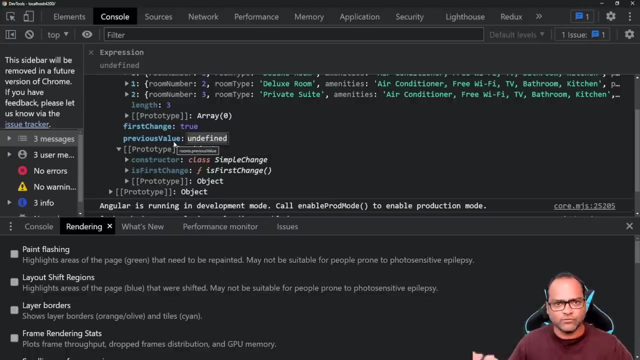 console log, which is here at the top, which says the previous value. you was like three records, and let me just refresh this right. so, uh, yeah, so you have current value three and then, uh, we have previous value undefined here. this is what i was looking at, because whenever your component is initialized, you will have of 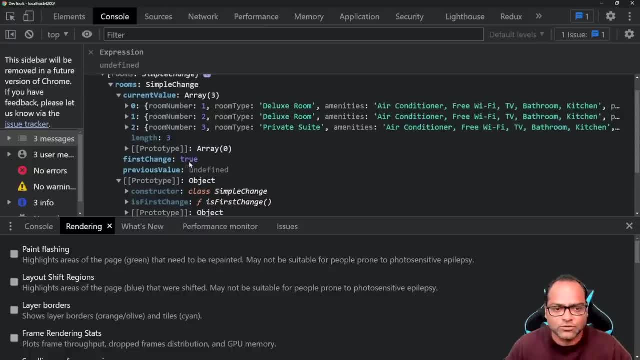 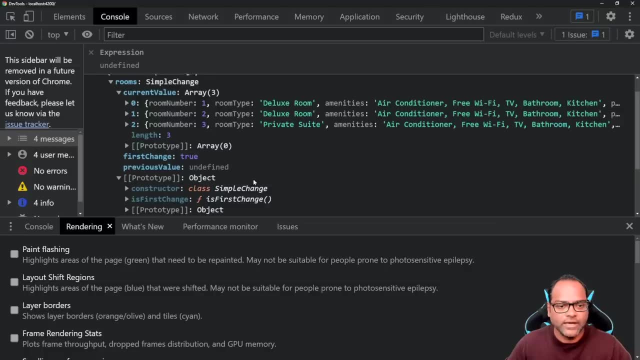 course, previous value will be undefined. and then you have first change as true, because this is the first time the value is getting changed, and then you have current value as three records and when i change it, every time you change this, uh, you will get the records available. 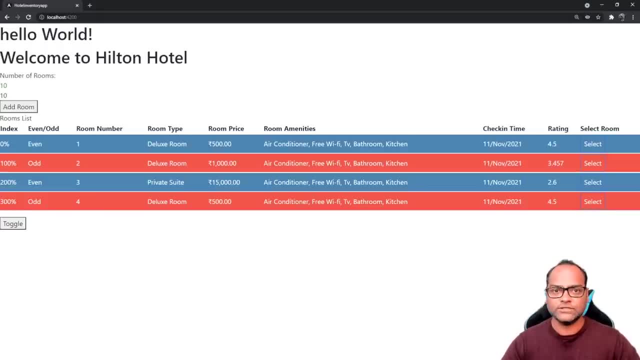 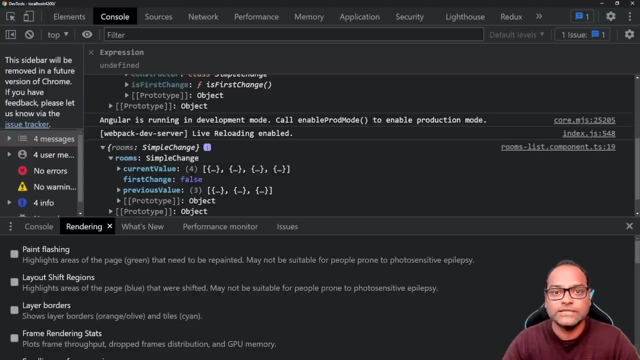 here now what is the use case, what where you can actually use it. so let's say, in case i want to modify some property after getting the input values, you can do it using ng on changes so you can assign it inside engine changes. but remember, ng on changes will only work in case you have. 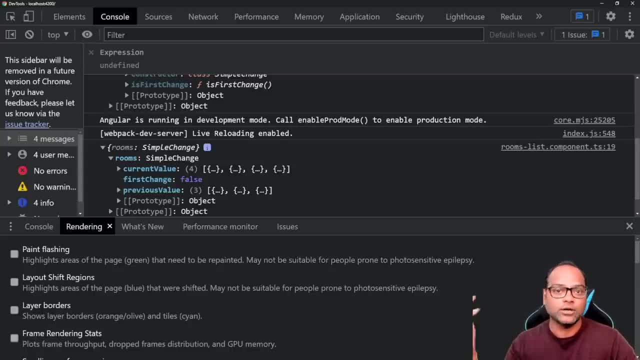 input properties and your input properties gets updated or you get a new value. remember this new value not updated. so it's like, whenever you get a new value, you will get, uh, the data inside ng on changes and based on that, in case you want to write some logic, you want to. 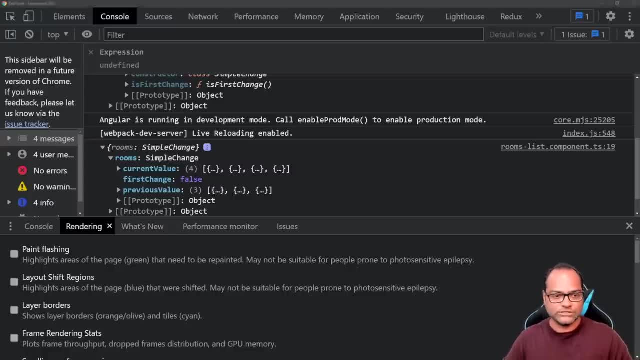 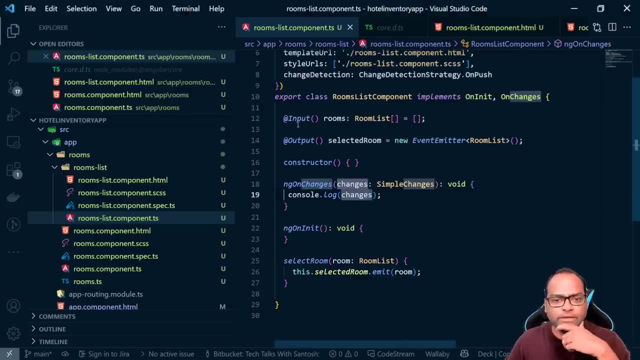 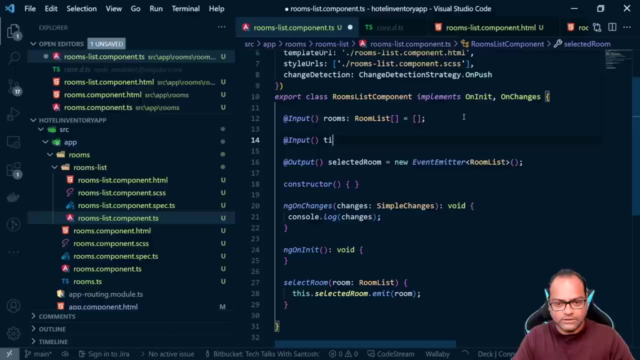 log these values. you can go ahead and do that using ng on changes, how you can access the properties. so let's talk about that as well. right now we have only one property called room list. i'll add one more property and we'll say this is title. and i'll say this is a type string and i'll say this: 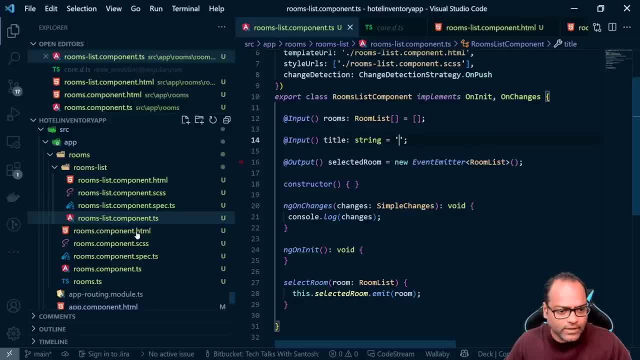 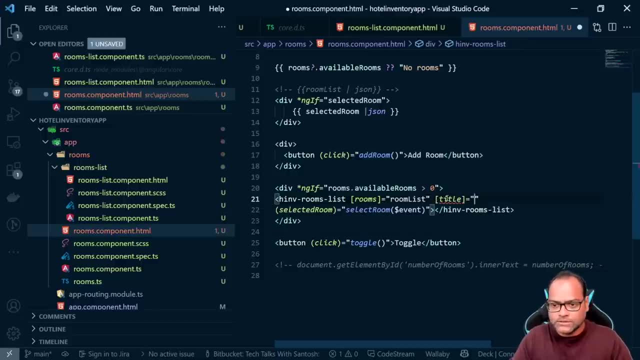 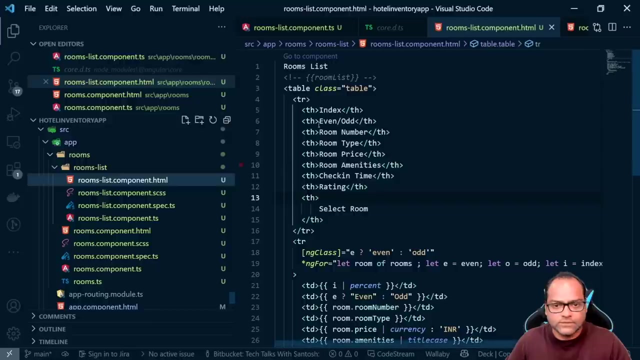 default value is blank. let's go ahead and try to pass this value as well. i'll say: this is rooms, and then we have our title is equals to room list and we want it to be in string, so i'll just use single quotes. so now it is string and let's find this value. this title is equals to rather than 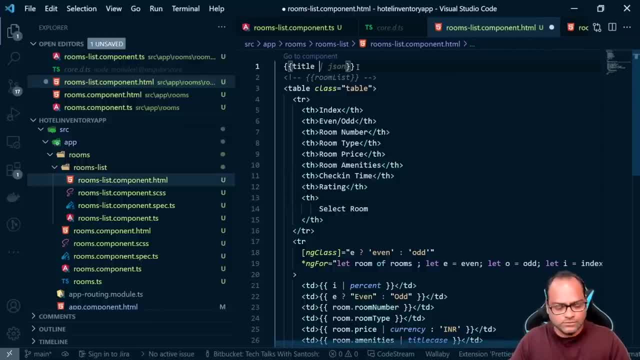 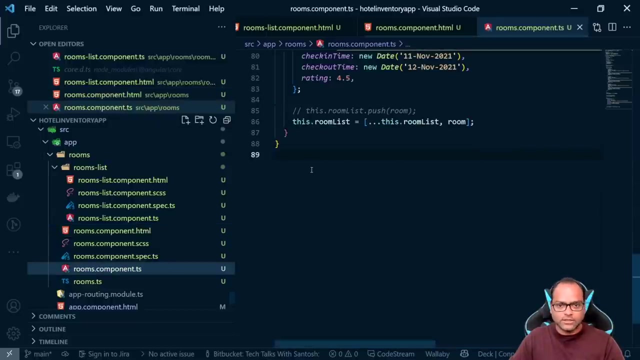 doing this. we'll see title here and we have rooms list available here, a room list available here, right? so just add, let's add- s2. okay, so we have room list, uh, which is coming from outside, so now let's go ahead and try to change this value, uh, and see what we get. so i'll just try it. another: 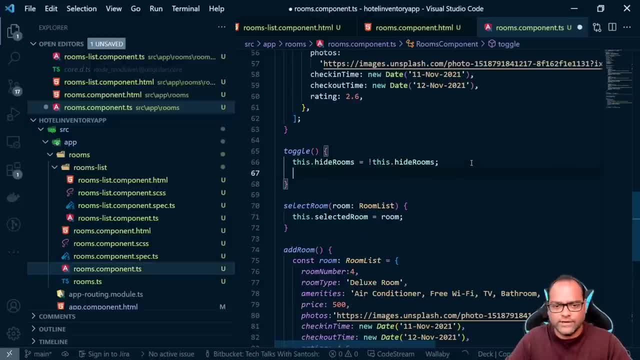 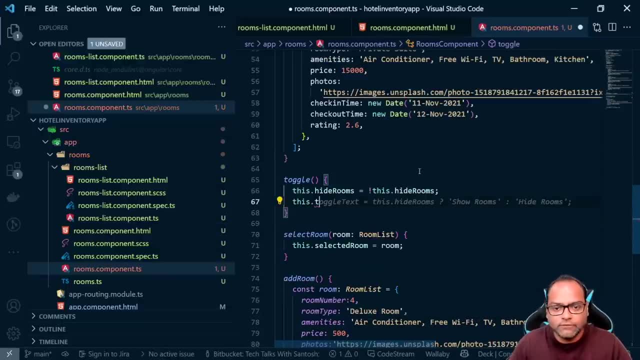 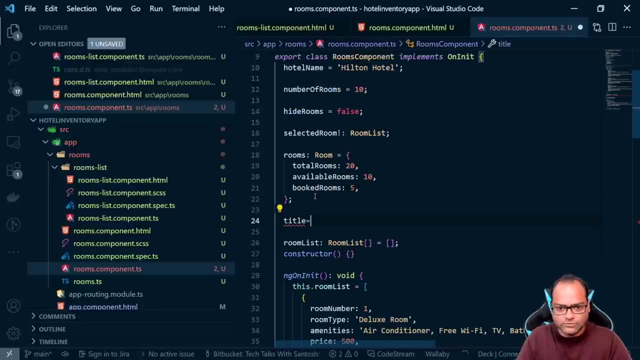 on click of the struggle button, right, so we already have the struggle button. i'll say this title, so we have. we have to define a тоб title property here. so i'll just say, okay, this is again. title equals to uh, room list and let's use this title property. 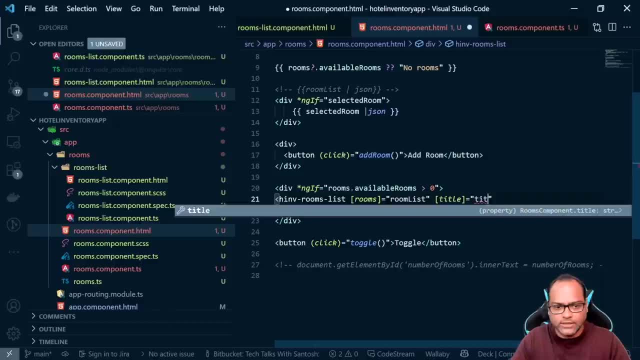 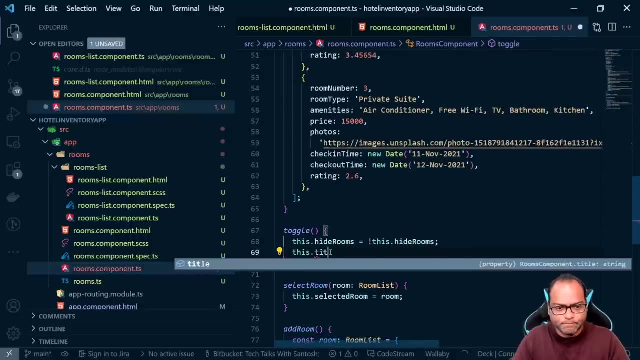 here now string. we'll just pass this title property here and on toggle i'll just change this to and say, rather than room list, let's call it as rooms list. and we just want to actually change the property and see what we get inside ng on changes and let's inspect. 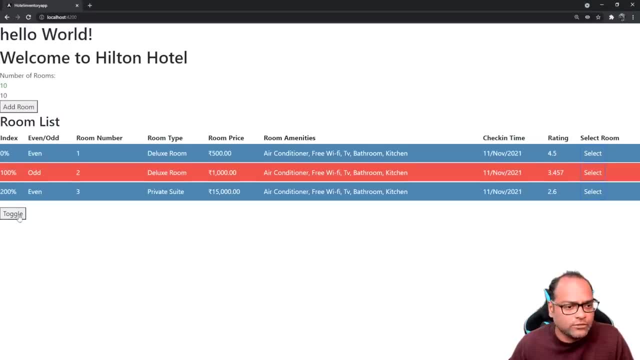 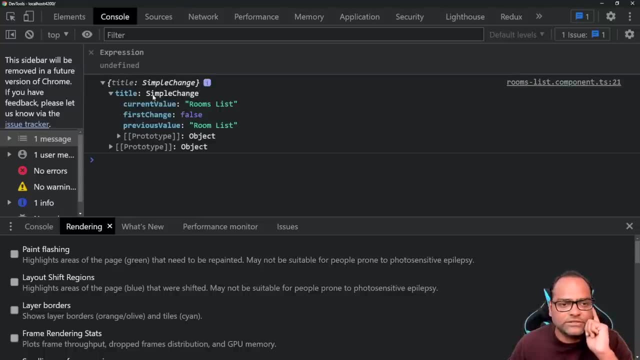 and let's clear this console and let's click on toggle and we have rooms list available here. so let's see what we get here. so you can see right now only the value which is which got changed is title right. so whenever you will change your input value, that will come as property. so here: 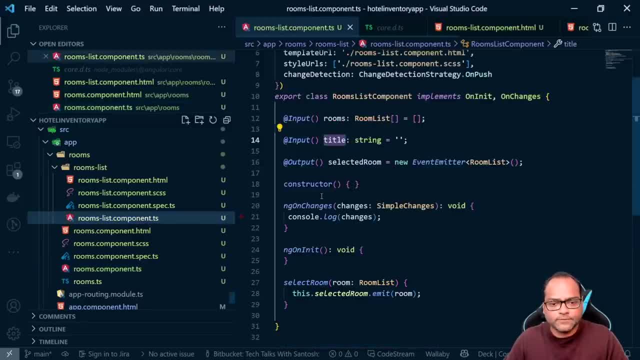 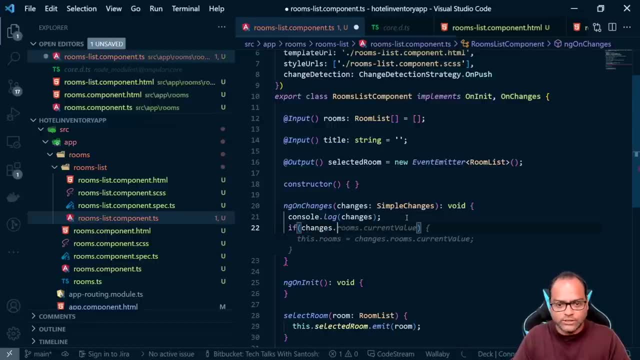 you can always do so. if changes dot, let's say title, which means the title is changed. okay, index signature. so i'm saying, if the title property has changed, so uh, you can do something like, for example: i can say this: dot title and changes dot title. dot current value let's apply to. 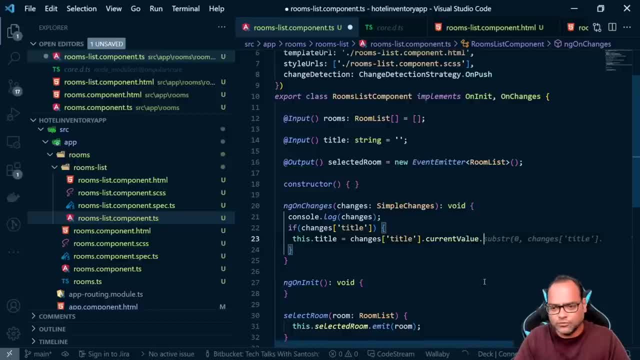 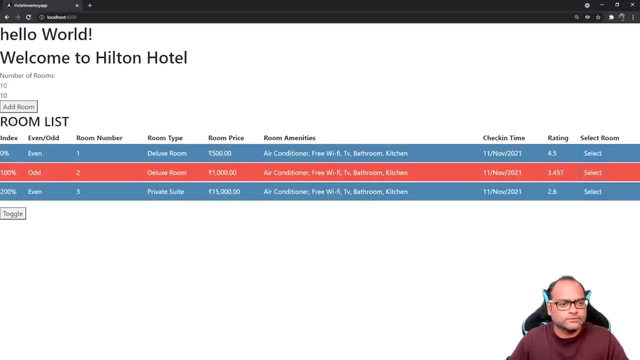 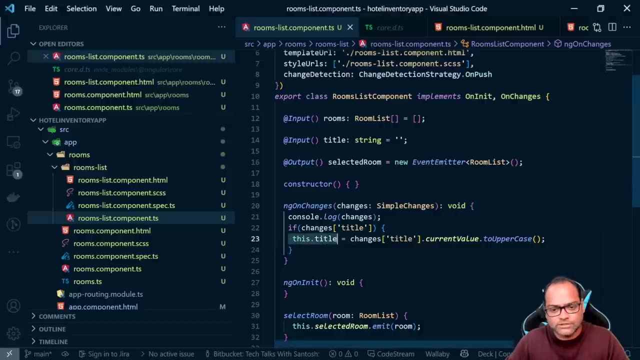 what we can do. let's try to do uh, the substring or to uppercase. let's. let's do uppercase current value, dot uppercase. you can see, uh, your property or value is updated to uppercase because of this and why it works, because, of course, here we are assigning a new value, right? so we are saying: 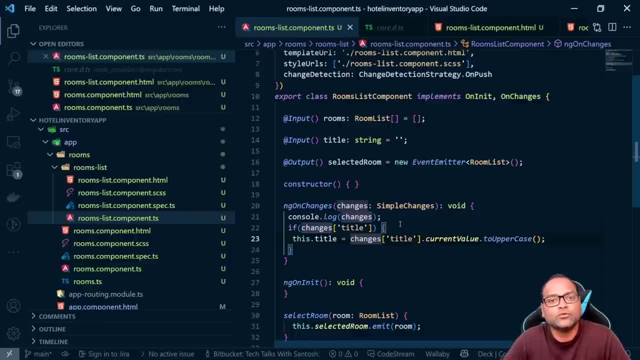 this dot title equals true. so this is uh, this is what you can do or achieve using ng. on changes, let's take a look. very useful in case you want to control what value needs to be updated whenever a new data is passed, or you want to run. you want to run change detection manually. that is also. 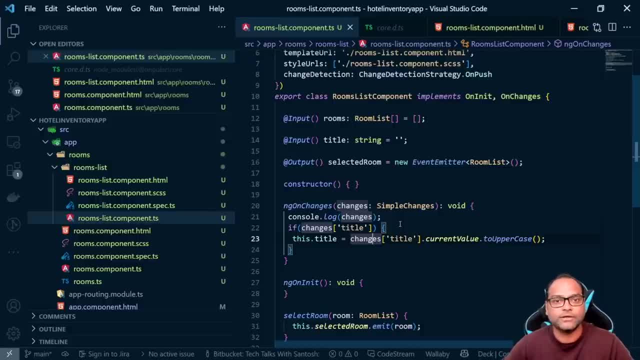 possible using this. probably we'll see once we talk about services, because we need to understand the services before we go ahead and use anything or any services available inside angular. so this is uh, this is it from engine changes. so what are the concept which we learned? because we learned about input and output. we saw how you can pass data between two components or 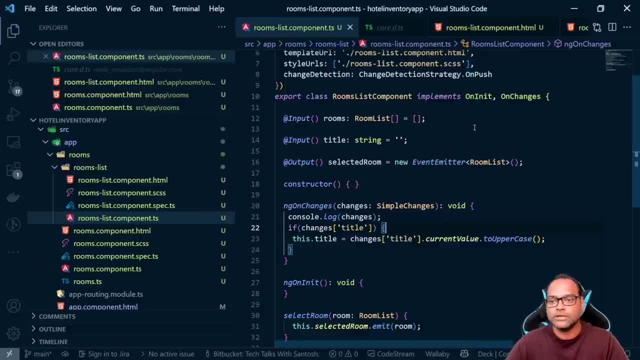 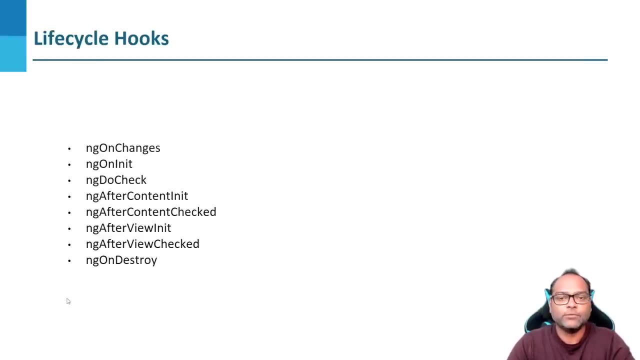 how you can do component communication using input and output. then we also learned about change detection strategy, which is really important. and then we learned about ng on changes. just because of engine changes. we have to actually learn these two concepts- very important now, as we have learned about ng on in it and ng on changes. and now let's move on to the next. 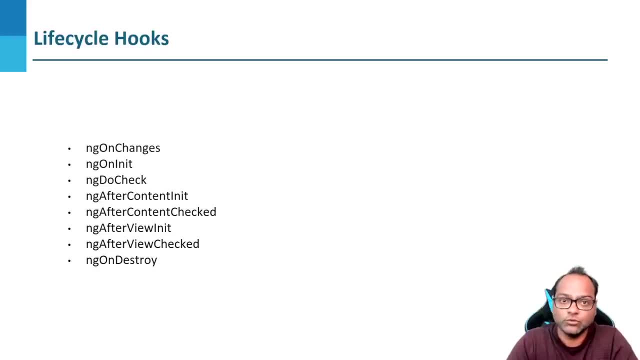 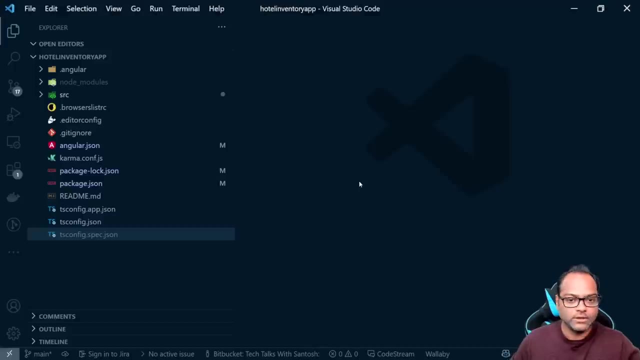 lifecycle look, which is ng do check. now, this lifecycle look is something which you will be hardly using, but you have to understand, or you have to know about what do check does. so let's go ahead and see it in action. so here, uh, i will just go ahead and add this on rooms componentjs. 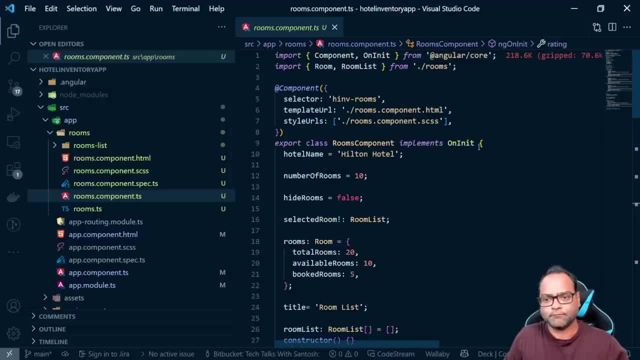 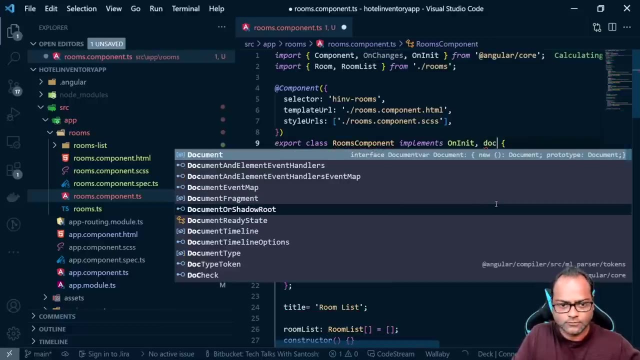 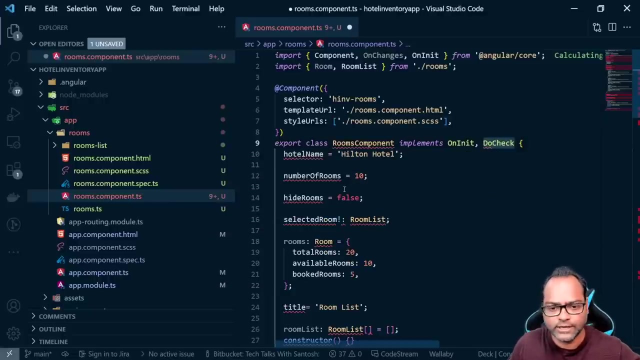 so let's go ahead and add this on rooms componentjs. so let's go ahead and add this on rooms componentjs. so here i'll say, okay, this is on sorry, check, yeah, so this is the interface which will be used for do check, and then we have to implement. 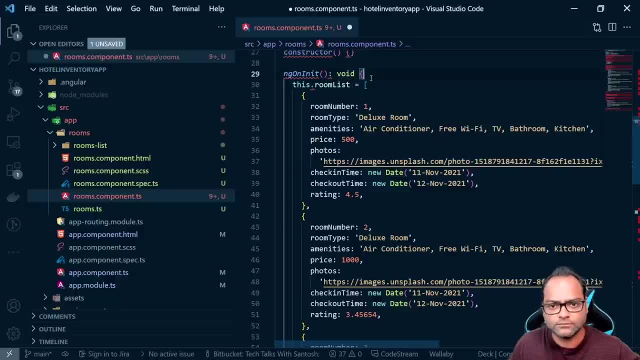 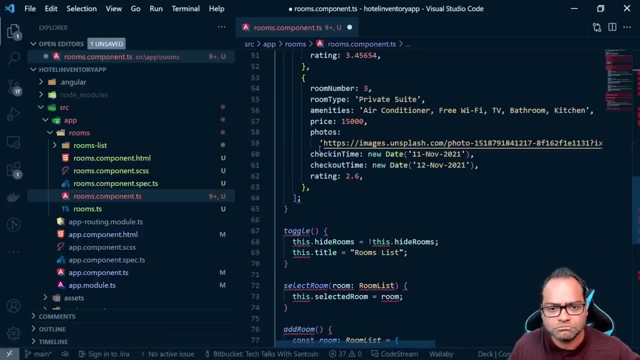 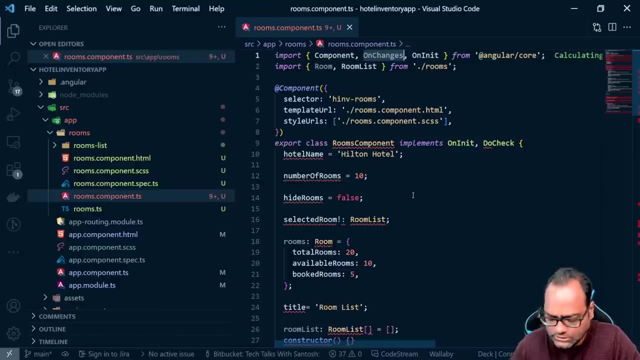 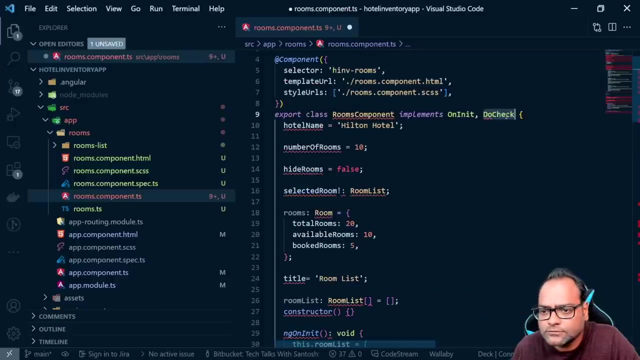 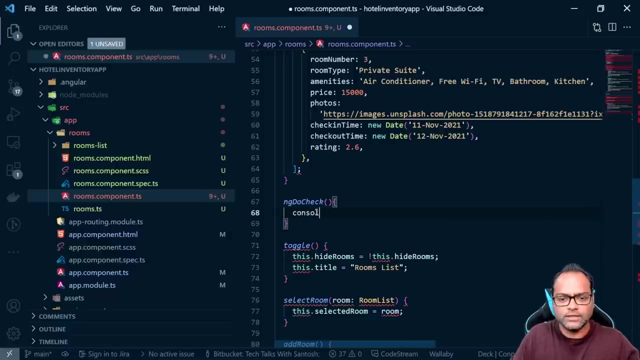 the interface and just okay, there's something wrong. and g do check and this is the method which we need to implement. so, on changes and remove this and we've gotten the consolelog site and now we arecom. malta is trying to do something which is we're trying to make too, but they can do something wrong. it should be what's. 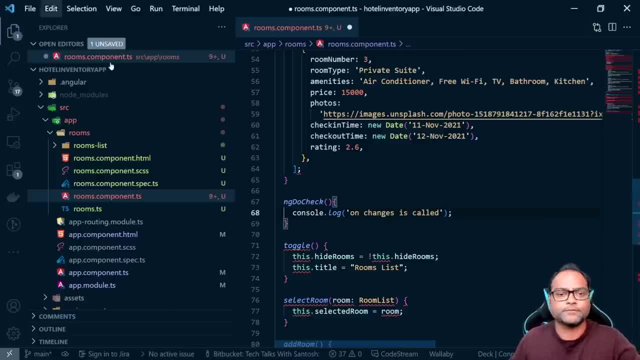 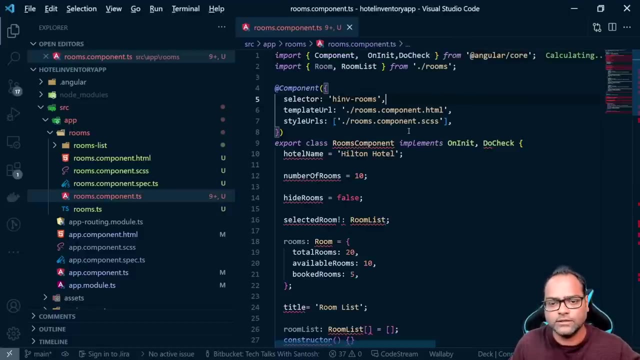 going to happen soon then. so in the show cancel, i will add this consolelog and here let's do consolelog right now. consoleloc and i'll say: on changes is already found them to chip, okay, uh, so let's add it on. on changes is called. 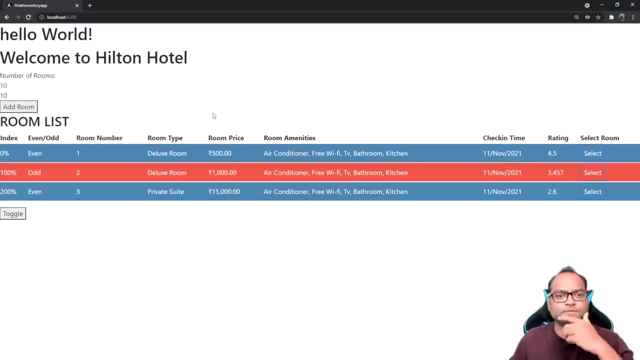 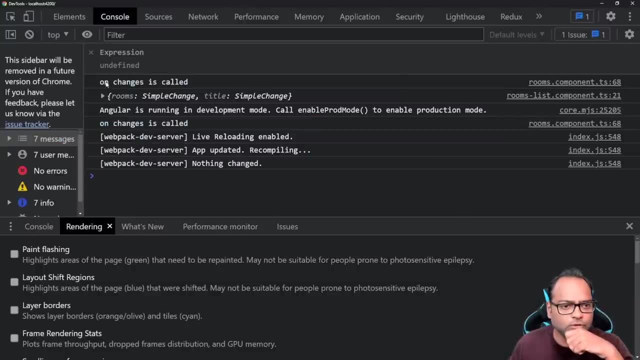 and it's completed. now let's go to the page and let's inspect the element. let's go to the dev tools and here on console you can see there is a message says all changes is called. now i'll just do one thing and keep it open here. 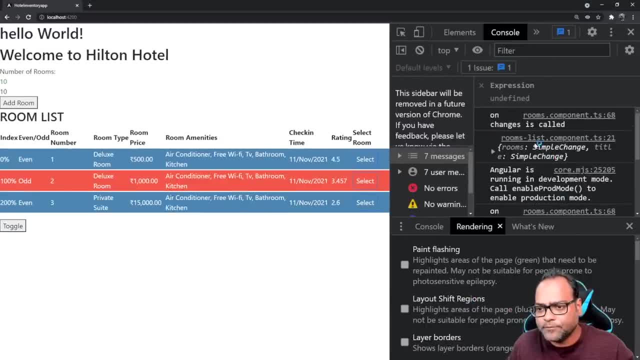 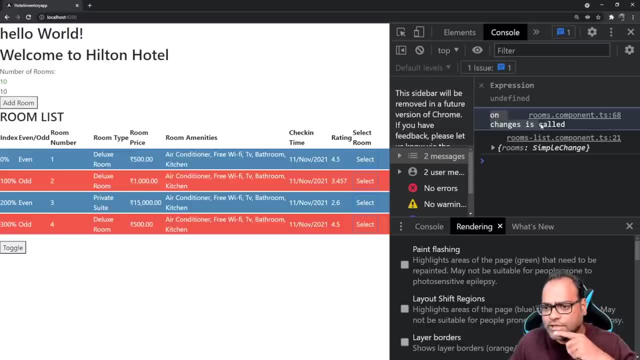 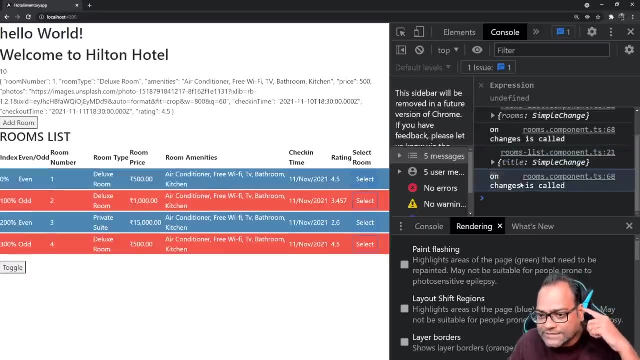 right, i'll remove everything and let's invoke some events. for example: add room: you can see on changes is called. let's click on toggle. you can see on changes is called you. uh, let's click on this select and you can see on changes is called. so what this? on changes event. 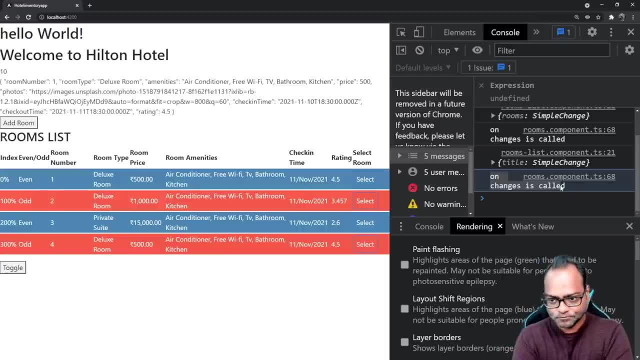 is so. this on changes event is something which will be executed every time you raise any event, irrespective of where you have it. this component is implemented or available. in case it is active, it will listen to any changes which has happened inside your entire application. remember that, so this event, uh, or implementing 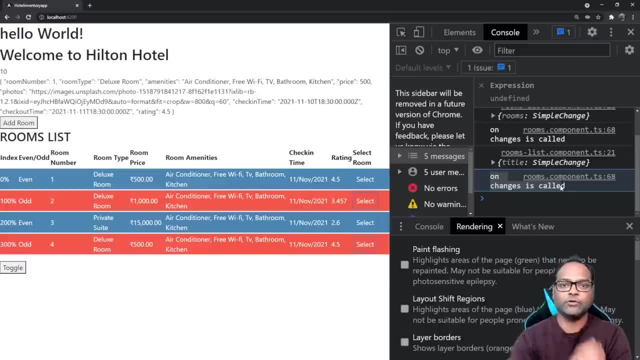 this lifecycle hook is very costly. in case, uh, what, what, what can be the use cases? uh for uh. in last four years, uh, i have been writing angular code and never see, never saw any example or any use cases where i had to go ahead and implement ng on changes. but it can be useful in case you want. 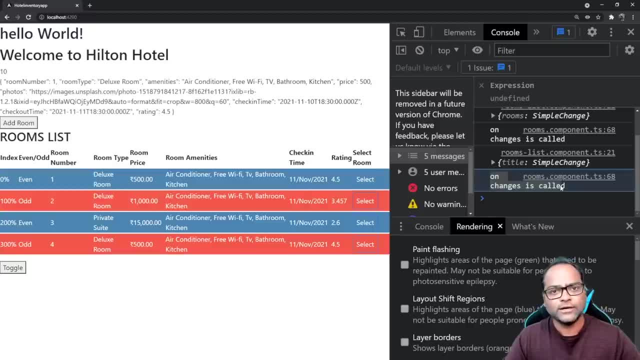 to detect some changes which is not controlled by anywhere. so let's say you have some logout button where some logout button plays on any some corner of your screen and you want to make sure whenever that log logout button is clicked you should go ahead and detect changes. but where you're not sure, 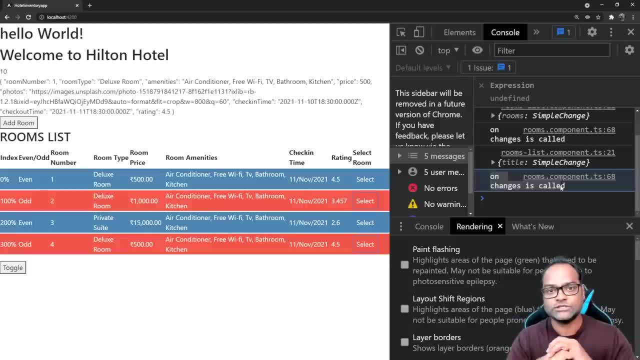 what you can do. what you can do is you can have any implementation of ng on changes or some not ng on changes do check event or do check lifecycle loop. as there's an event which is raised, do check will be called and you can handle your special scenario where, of course, that event 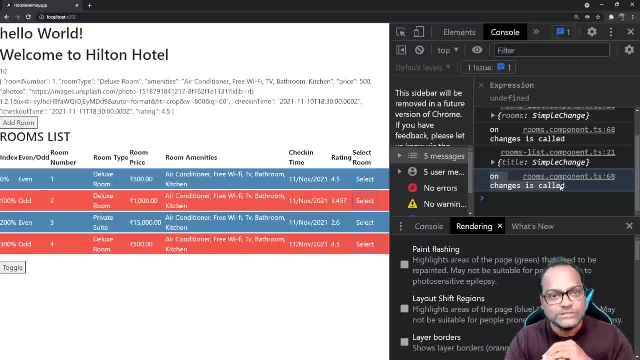 is something which is not captured by anyone will be captured by your. do check lifecycle loop. so that's uh one you. that can be one use case, but try to avoid it as much as possible. also, another thing which you should keep in mind is you should not implement ng on changes and do check together. 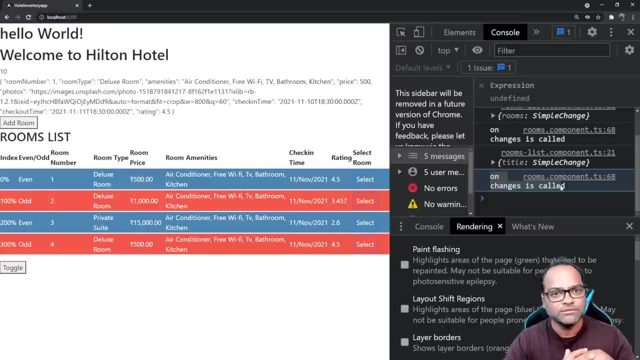 on same component, the reason being, of course, both are going to do the same thing. what on changes does? it will detect any changes to your input values. what changes on do check will do? it will detect any changes inside your application. so it will be like capture twice. so don't do that. 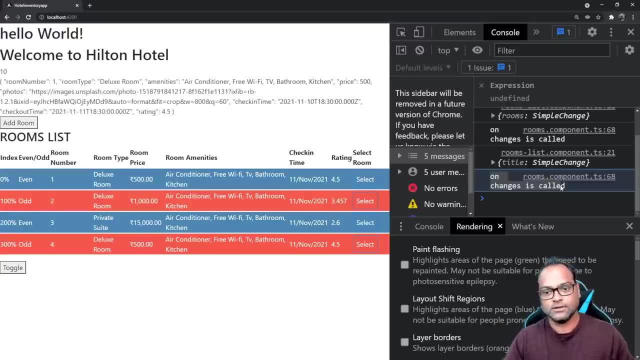 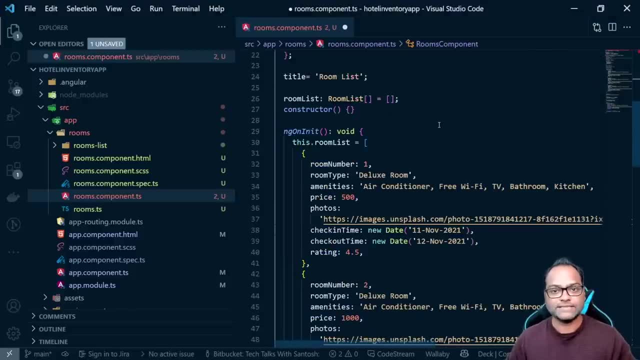 and try to avoid. on changes: sorry, do check as much as possible, not on changes. to check as much as possible- uh, some i like external changes. do check as much as possible. uh, some like external changes, extreme use cases. if you get into it even before doing that, just try to in case you have some. 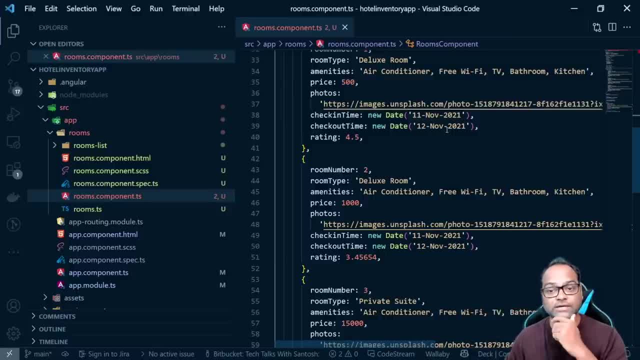 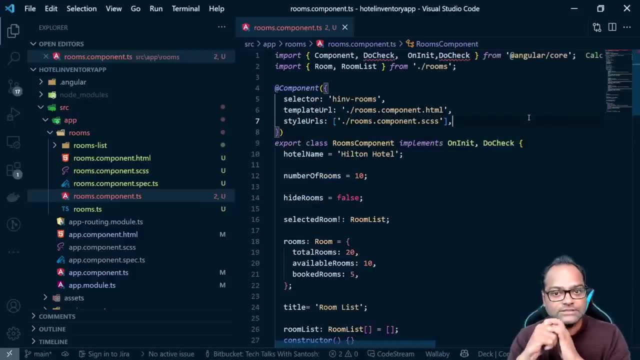 special scenario where you think that do check is some do check is the answer. uh, you need to implement do check. i would suggest go ahead and check on stack workflow, ask, ask the question if what you are trying to do is correct and then use it otherwise don't. so this is ng do check. 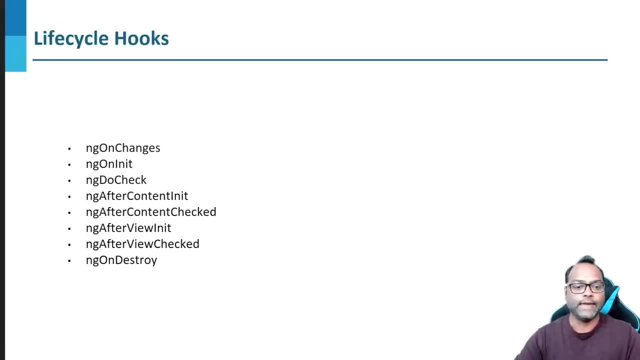 in this video we are going to discuss about ng after unit and and ng after we chat, and we will also discuss about something known as view child, and we will learn about some other stuff like template ref and how you can dynamically load a component. so let's go ahead and get started. so far, we have discussed about on 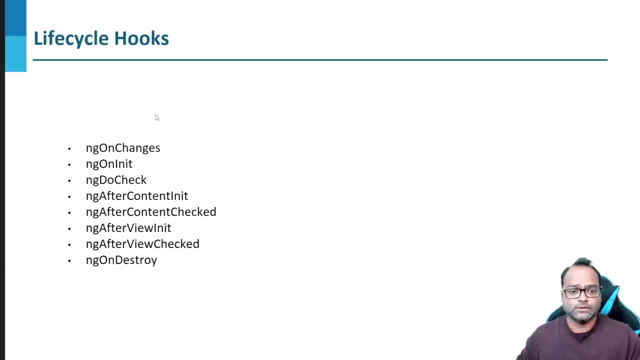 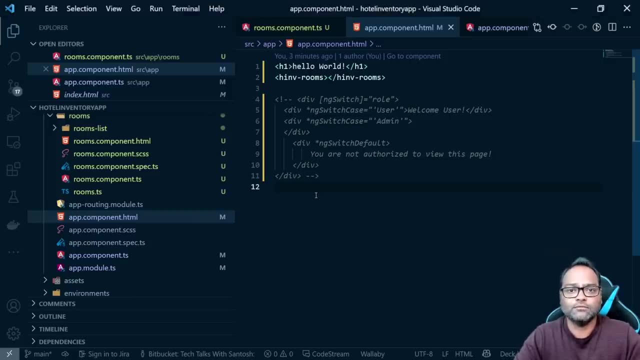 changes on it, on in it and do check so to understand how you can actually use ng after unit, we have to first learn about view child and how we can actually communicate or load a component using viewer child and what else we can use, uh do, using view child. so 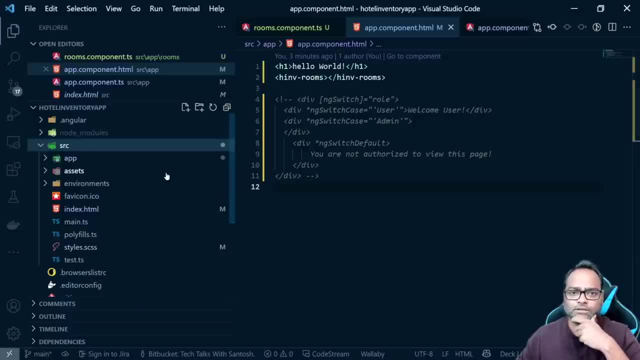 let's go ahead and do that. so we'll start with a simple example, the first example, which is, which is really useful. you will get into a lot of scenarios where this may be helpful for you, but i want to review- i've done some work on this as well, of course, and the to do cycle something all the time, but i want to see what it does, so i'll have to discuss it at this point, in this state. so for now, if you would呢. 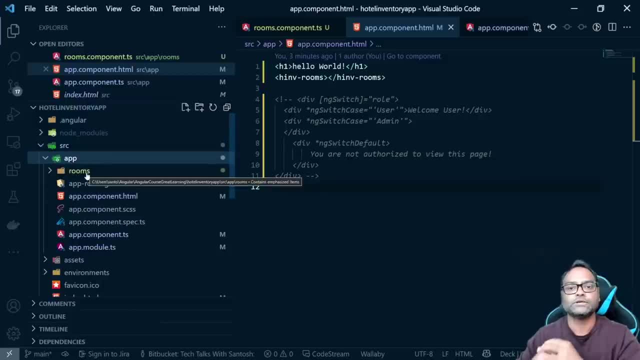 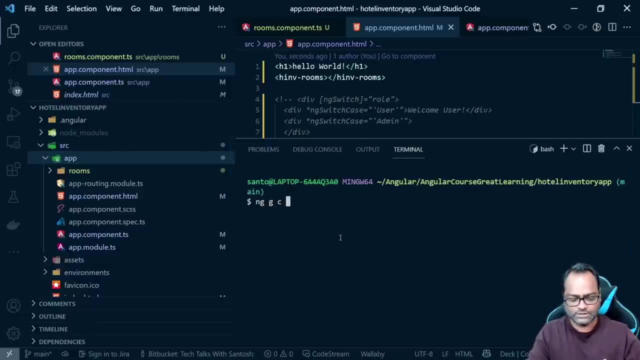 you. so let's go ahead and do that. so what I'm going to do is I am going to create a new component and we will communicate to that component using view child. so I'll call this component as let's call it as header component. so let's say nggc and header. 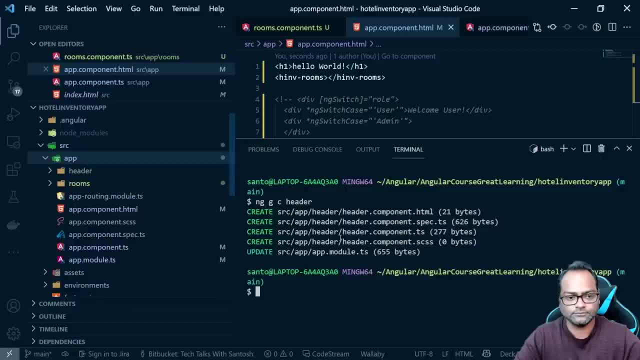 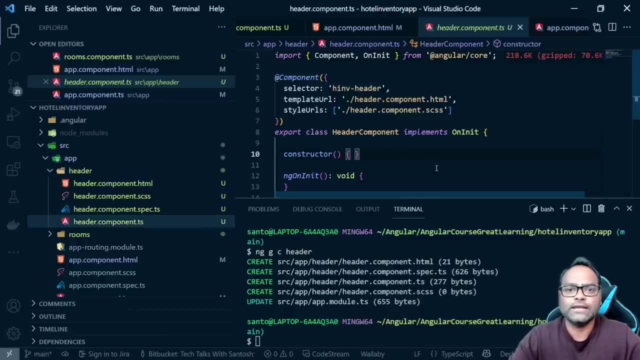 now we have already seen an example where we have we are actually communicating with a component which has input property and then the child component can send some data back using output. so in using input and output. but this is another way. let's say, you have a component, but 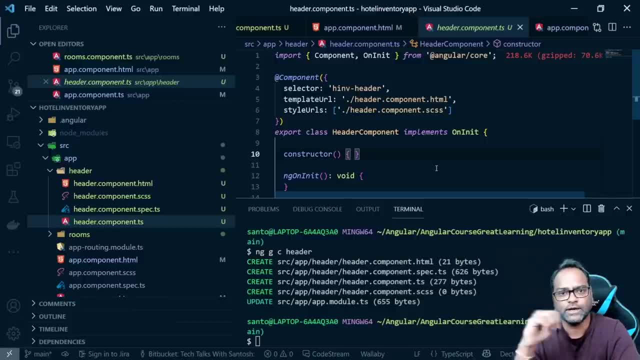 you don't want to actually make it reusable. I mean you don't have to, don't want to actually have input and output properties because most of the time they will be individual component. but sometime, let's say, you may need to load them in another component. you may want to access them in another component and probably assign some property or call some. 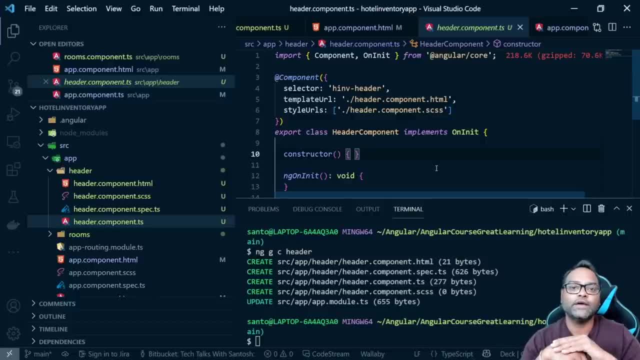 function of this particular component. or let's say, you have any third-party component- this is really a good use case for viewchild as well. so let's say, you have a very third-party component which on which you don't have much control, right? so it's like they have some component and then 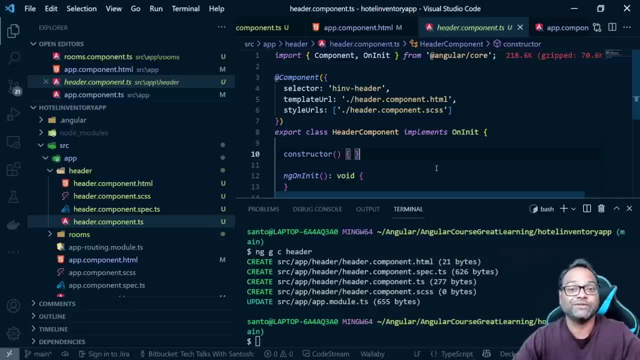 you can pass input and output properties. or let's say they have some component where they don't- let's say you get an library- ui library- and where they have some component which is internal to them. so they don't want to actually make it reusable, but maybe you want access to that particular. 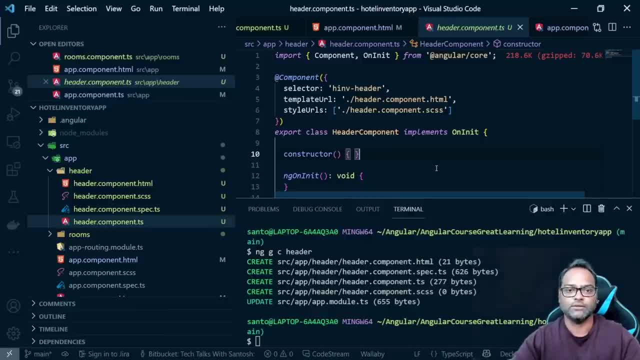 component. you are working within a team, like multiple projects working together, and it's a library, so they they don't want to make it reusable like using input and output, but you may want to actually access them. so what? what are the approach? what is the approach you will take? of course, you can go ahead and talk to the team and ask them to make. 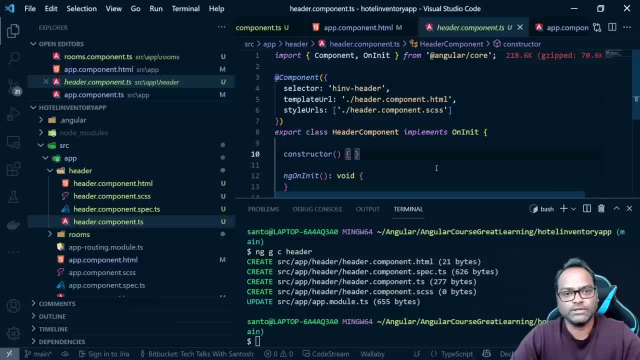 it reusable. but let's say they don't want to do that, right, i mean, it doesn't fit or it doesn't actually help in their use case. so what you? let's see how we can actually do that, how we can actually access any component into other component which doesn't have input and output property. 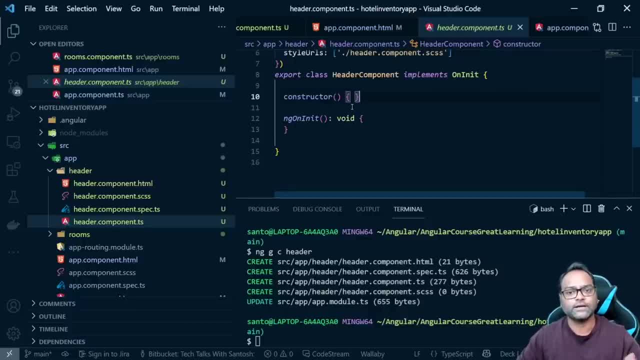 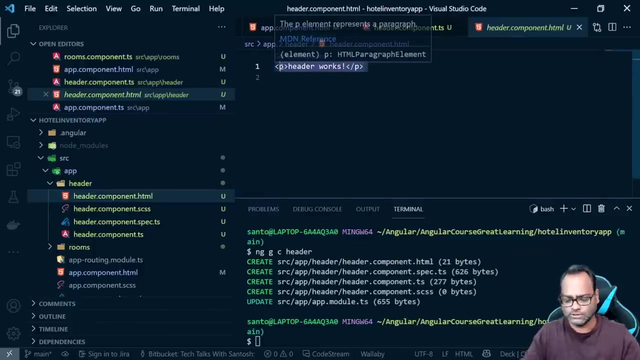 so let's create. so we have already this header component. now what we will do is we will create a property here and remember, i'm not going to make it, make it a input property, okay. okay, so we have title which is of type string, and i'll put this title: 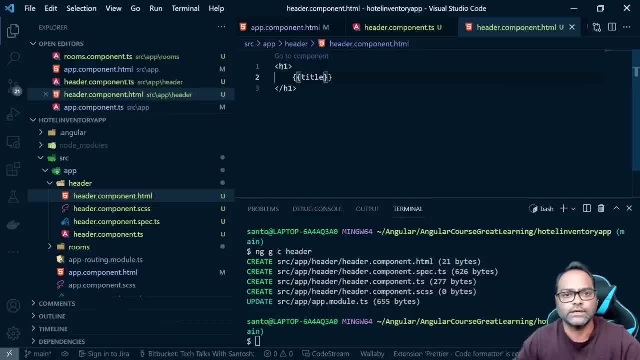 here using interpolation syntax. so far, so good. i mean, you created a title and you don't have to go any further so you can actually create another component here, and so that's the important thing. good, i mean, you created a new component, you assigned a new property, and then we just added: 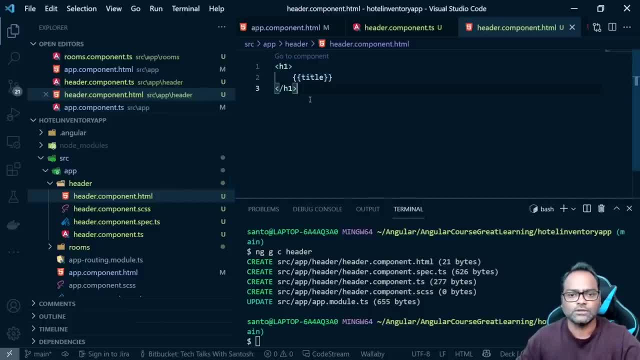 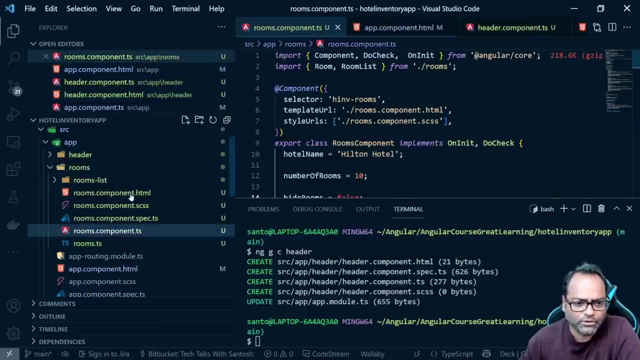 that into our interpolation syntax. so we just added that into our interpolation using interpolation pollution syntax. sorry, we just added that using interpolation syntax. now let's go to app, component dot html, and let's say: or let's go to room, component dot. html. so we have this welcome. 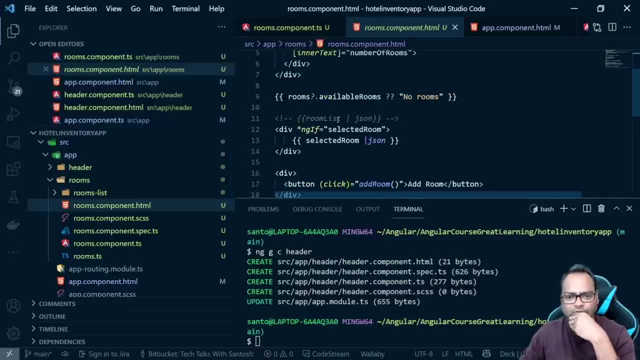 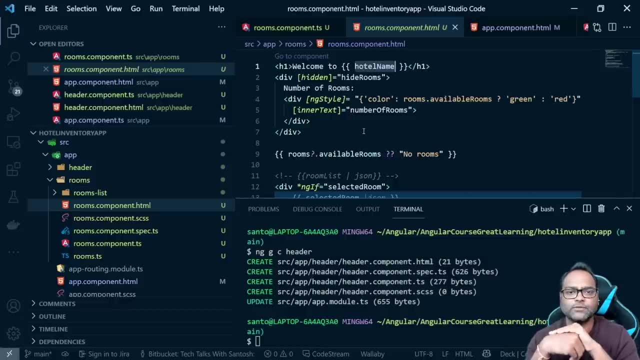 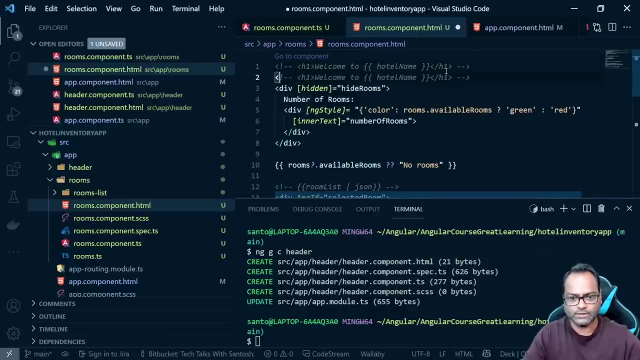 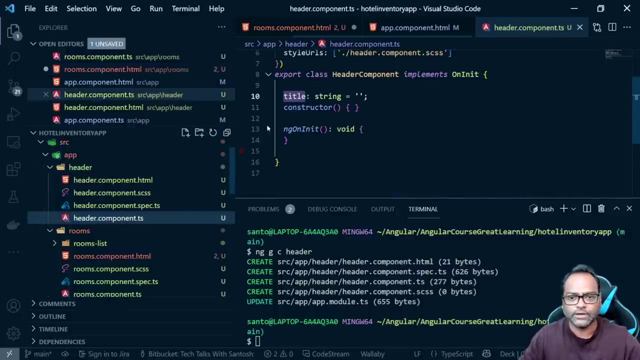 to hotel name. uh, what we want to do is we want to have an title here and we want to use this header component. so let's see how we, how we do that. so i'll just comment this out and we will use the hotel header. is that the component name? oh, sorry, directive name, no, so this is the directive name. 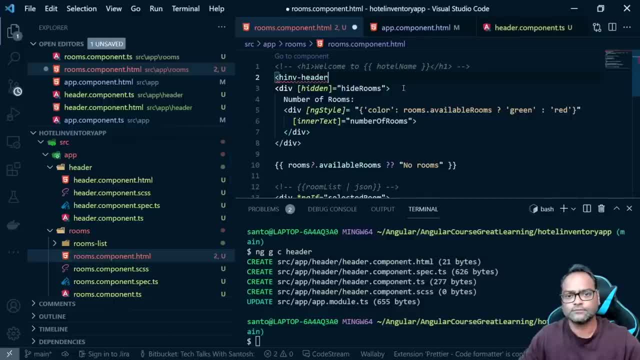 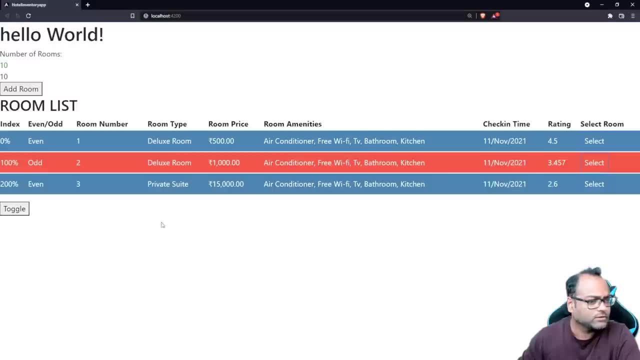 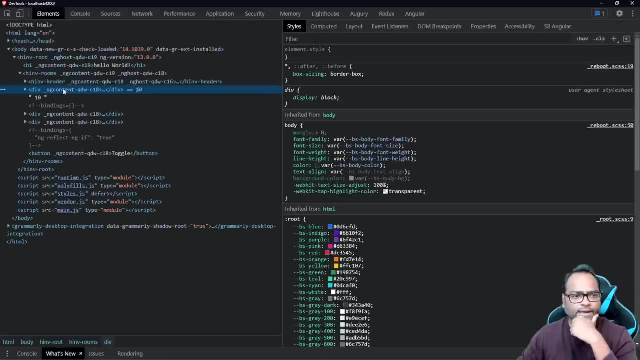 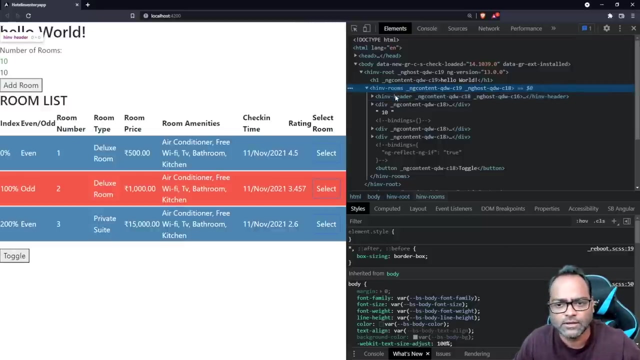 and this is it. so we have placed this component. let's see how it looks like on ui. okay, so we don't have that particular h1 available here, so let's inspect and here let's open it here. so you, uh, we have this header here, but i mean 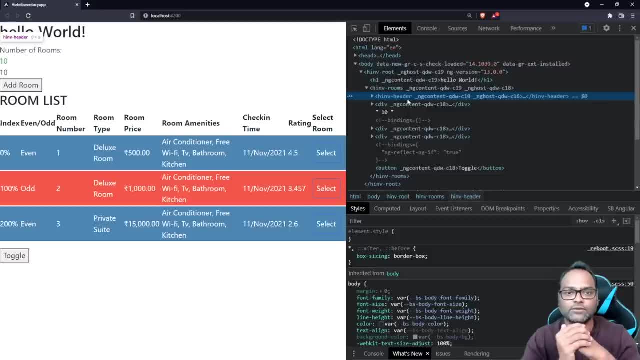 we don't have any property right, because how to pass the title now? i mean, that component is uh, that component doesn't have input property, it just have a property. but what in case? i want to access it now. let's see how we can achieve that using viewchild. 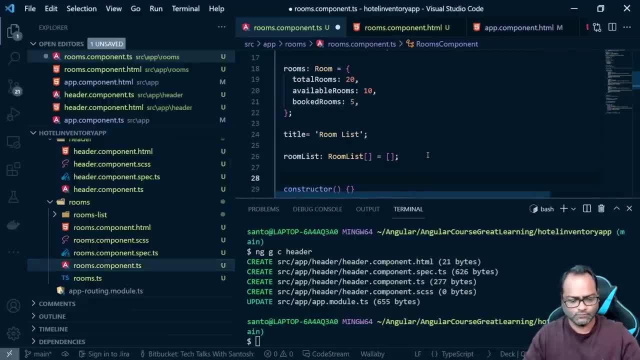 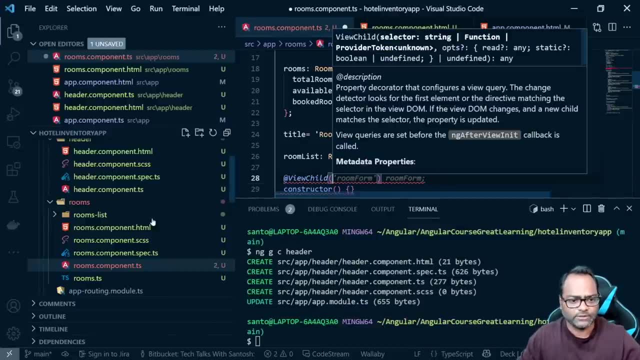 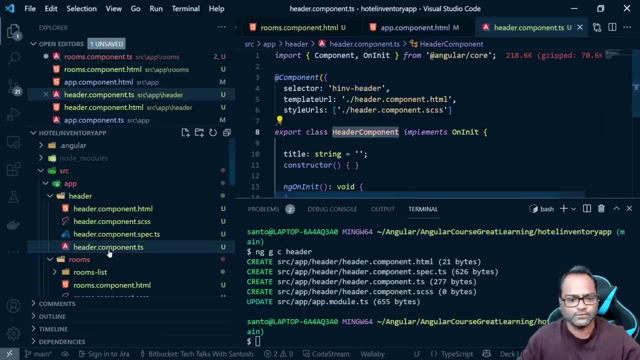 so here we will create, we will use viewchild- it's a decorator, so virtual decorator- and then, uh, we need to pass some parameter and we'll talk about that parameter as well here. i'll go ahead and pass this component, which is header component, right? so this is the component we want to access. 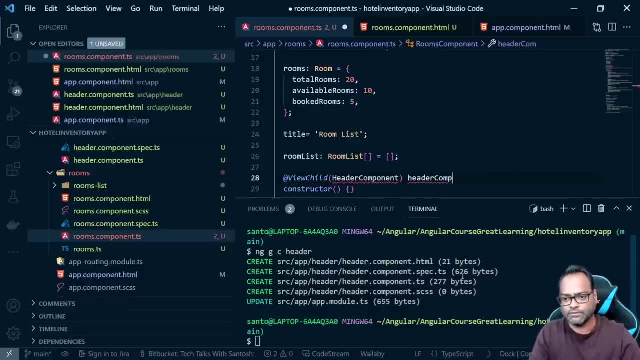 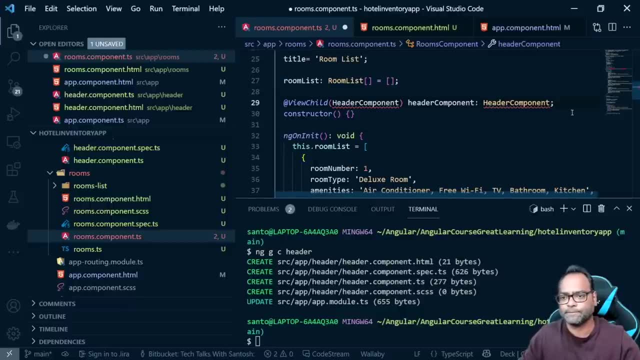 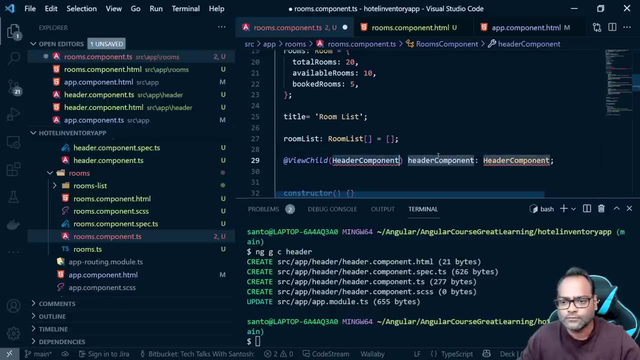 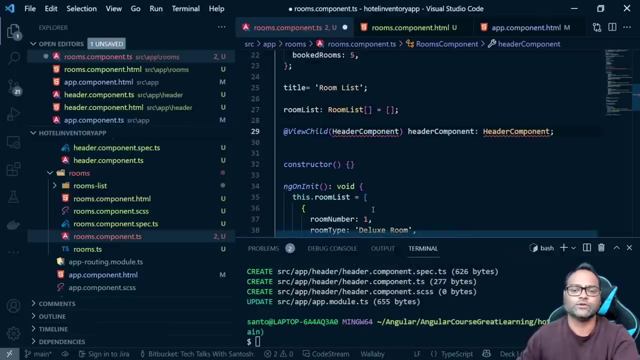 and i'll call it as so. this is a variable. i'm saying: this is header component, of type header component and let's import this header component. in this case, we will use this one for some reason. okay, we have already imported other components. somehow. editor is taking some time, for some reason, anyways. so what we did here? so using viewchild, what 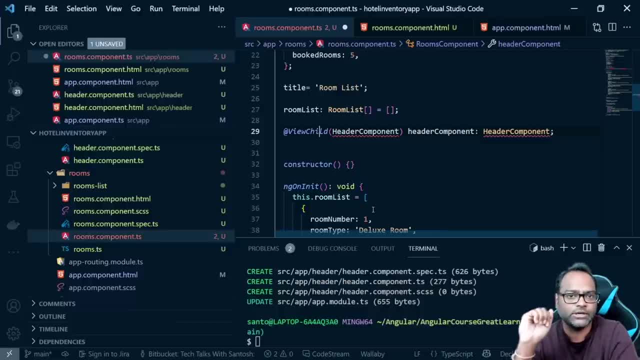 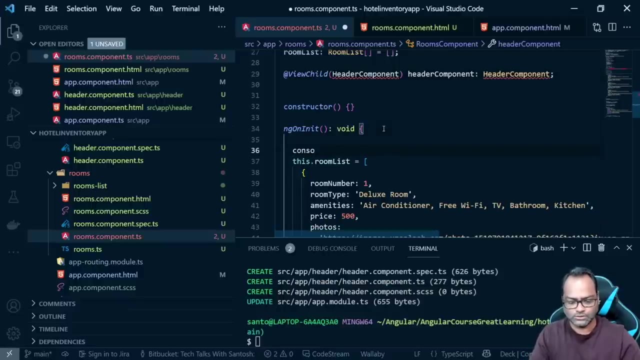 we have done is we have created a new instance of header, this header component, and we can access this instance inside this component, inside the rooms component, right now, so i can access any property, achieve whatever i want to. but there is a catch. let's do console dot log here. 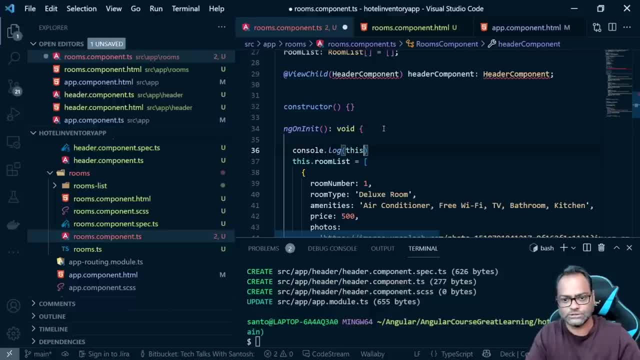 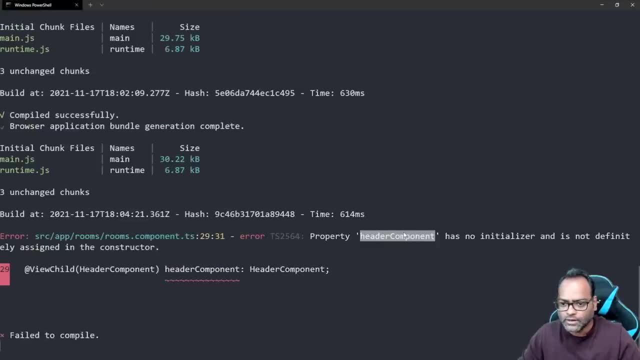 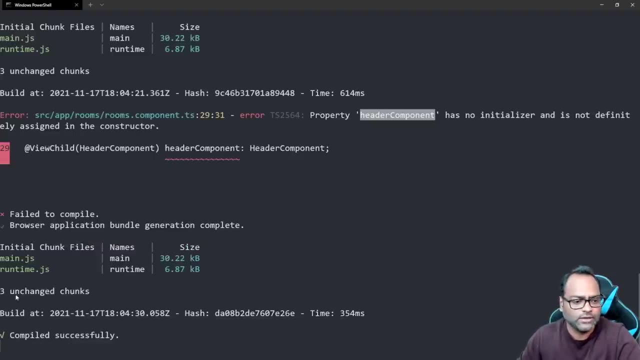 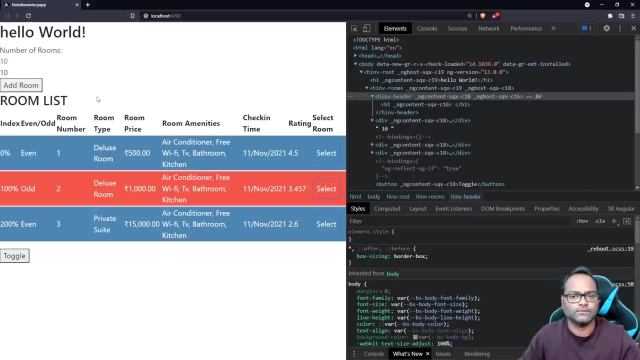 okay, somehow my indelicence start stopped working. let me just check. so this dot header component has no initial answer. okay, we are using script mode, so i'll just put this question mark to avoid this particular level. and it is compiled. let's see the output. let's see the output now. so we have. uh, let's go to console and here: 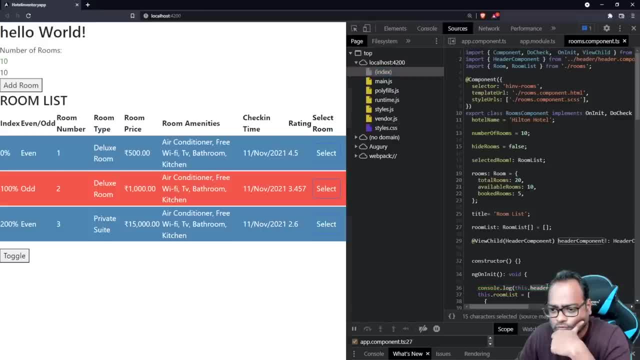 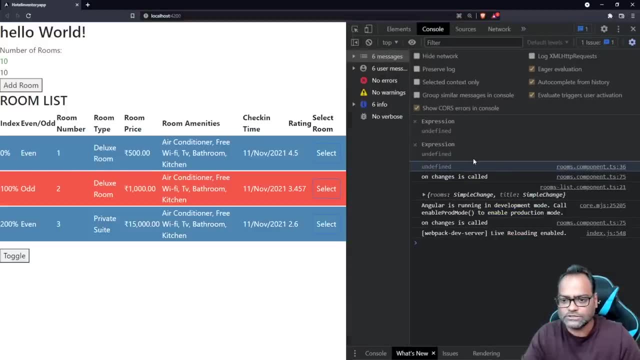 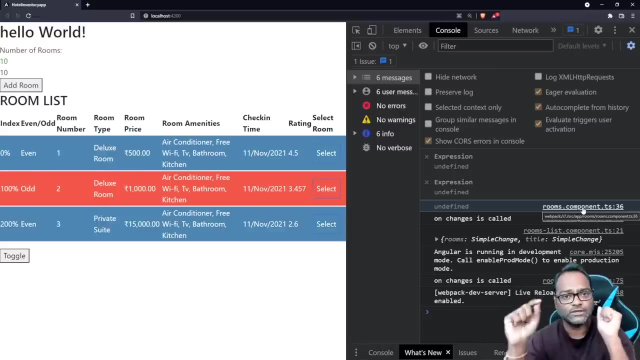 rooms. component ds, line number 36: yeah, here, so you can see. uh, what we have available here is- let me just zoom in- we have undefined these, as i i specifically said that using view child, what we are doing is we are creating a new instance of this particular component, but why don't we have anything if it's a component? i mean. 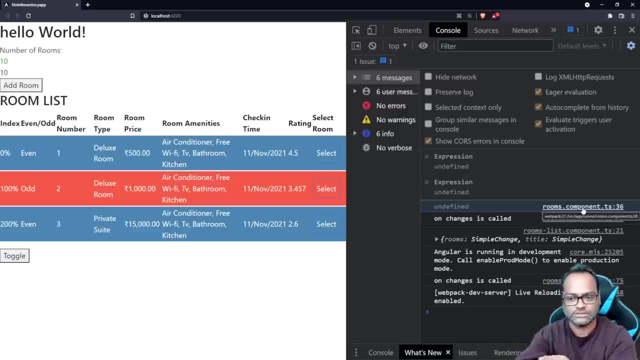 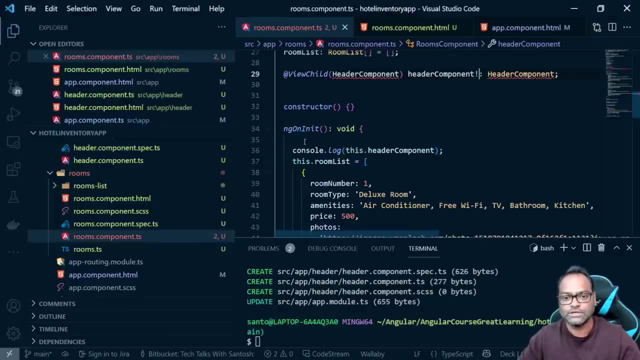 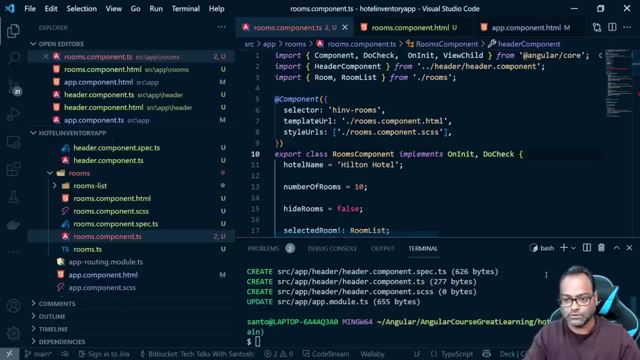 it should give us some metadata information right about that particular instance, but we don't have here, so let's see uh, why and how we can access it. so first thing which i'm going to do is i'm going to create our, i'm going to implement after view, init in. so let's go ahead and do that. 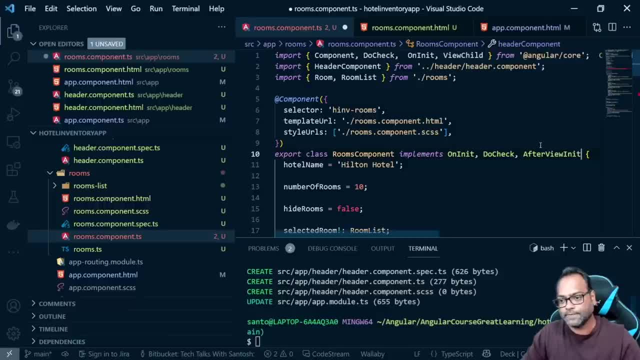 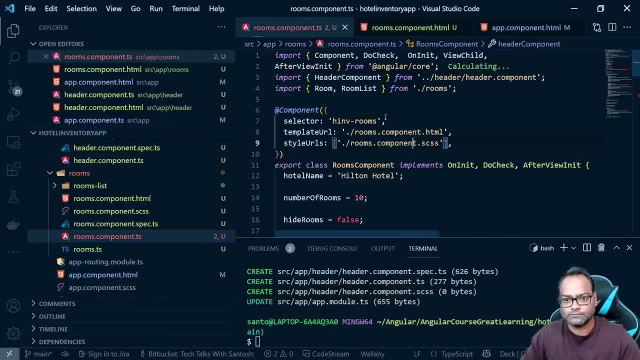 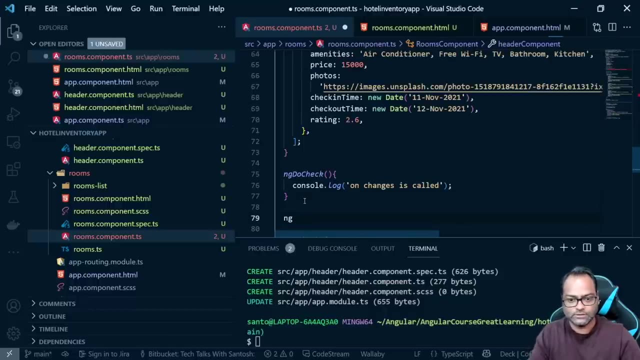 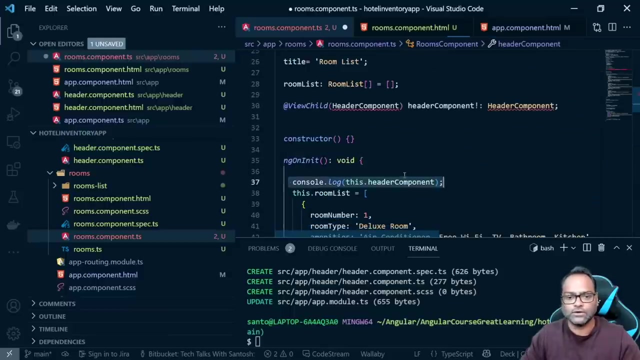 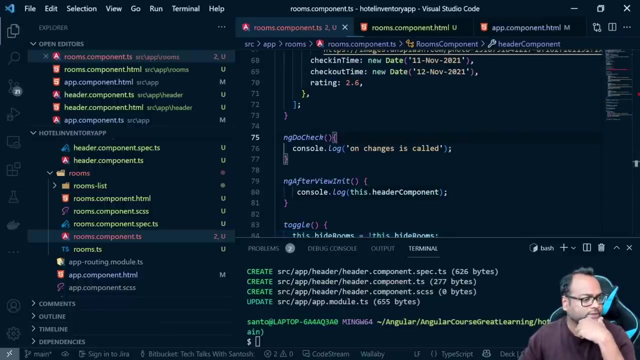 after view in it and we'll implement the interface, which is ng after variance. and let's use the same line which we have written here on line number 37 and let's test it on line number 80.. this saved, so let's go ahead and see. and it is simply, it is compiled successfully. and now let's. 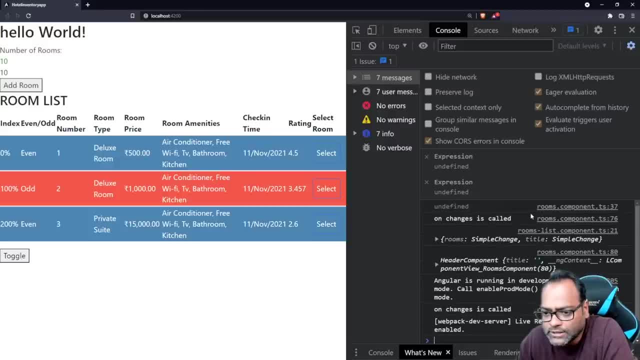 go ahead and see so. on line number uh 36. sorry, now line number 37, as i added one more line- we don't have anything we still have undefined. but at line number 80 we have the same instance but we have now some metadata. so what is that metadata? it is giving me information about. it is giving me 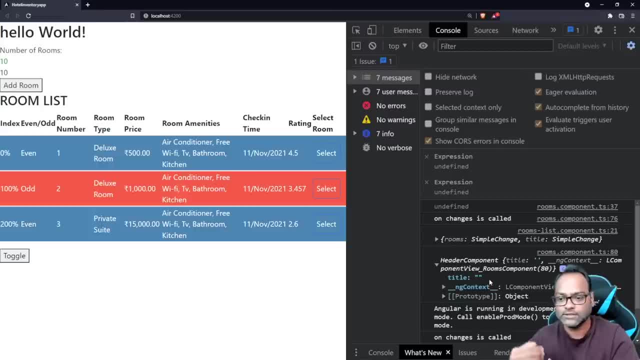 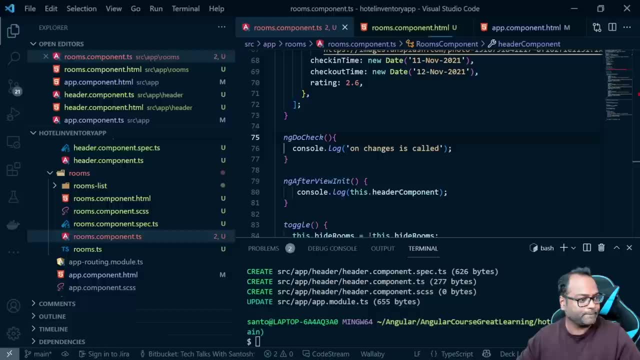 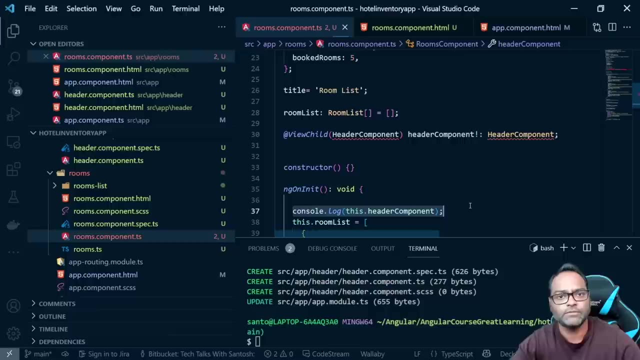 information about the header component. so i just said that it is going to create a new instance, and it is. it has created, but this instance is actually available inside after unit, not inside ng on in it. why so? so let's uh discuss the difference here. using view child, you create a new instance, but there is one more property which you have to. 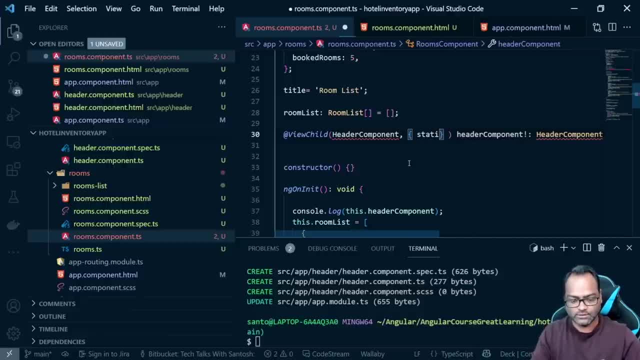 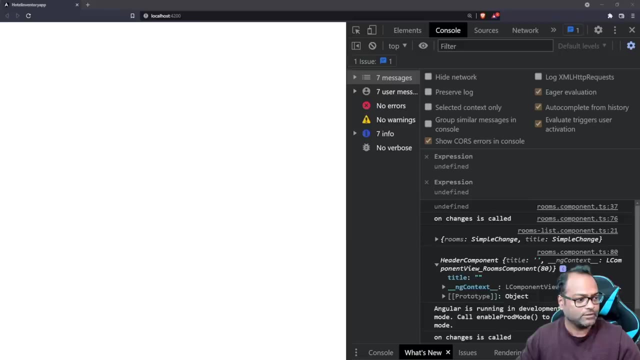 provide here. let's uh, do that and we will discuss about it. so there is a property called static true. by default, this static property is false, and what happens when we make it true? so let's go ahead and see both in the inaction now. you can see: now, after making static to true, I started getting 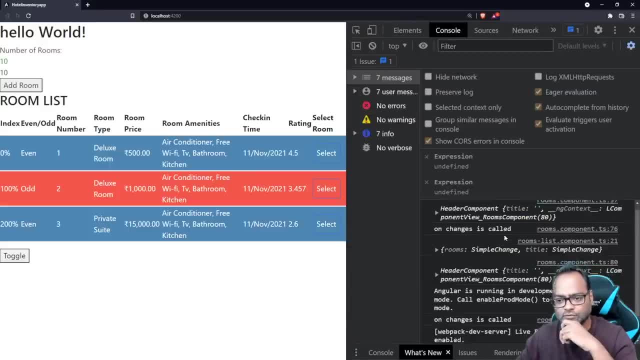 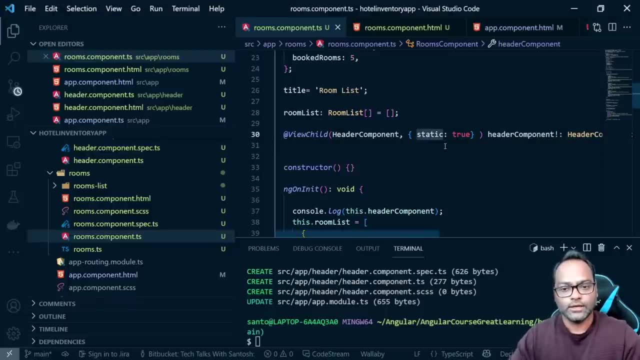 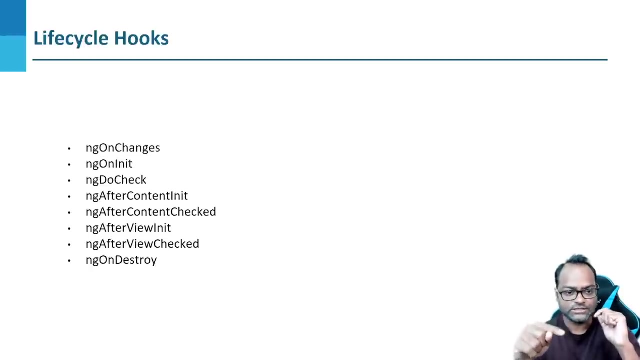 an instance at line number 37 and of course, I will get an instance at line number 80 as well, because it's a little so. what we achieve using static to this is here, you, where you have to understand the component lifecycle book properly. let's go to the slide. so, if you see this life cycle, look engine changes and you. 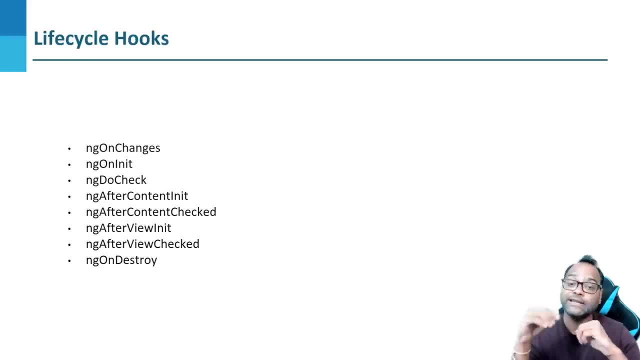 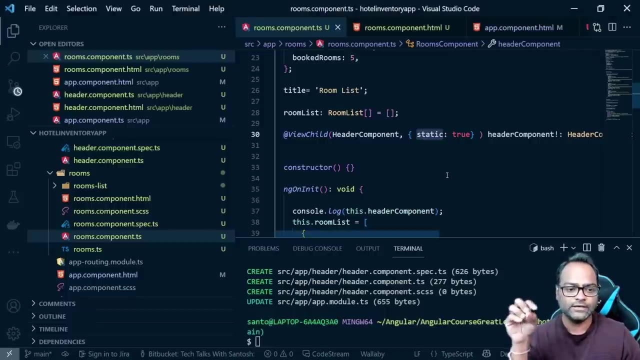 need and you to check, and then we have content in it, content check, and then we have after unit and after view checked, and then same and G on this one. this life cycle will execute for each and every component. now I am right right now: inside rooms component. 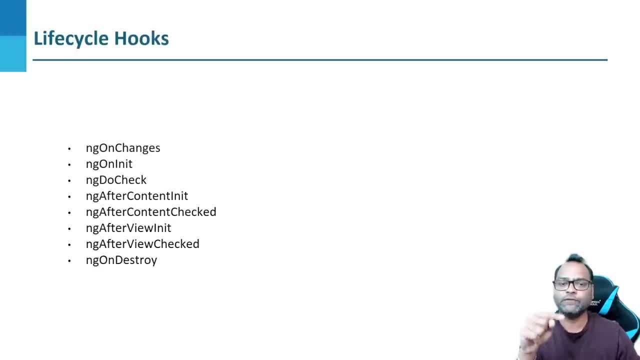 What I'm trying to load. I'm trying to load header component. So what will happen here? So let's go through it. First, the ngOnInit of your rooms component will be called, and then, after doCheck, after contentInit, after contentChecked, after viewInit. 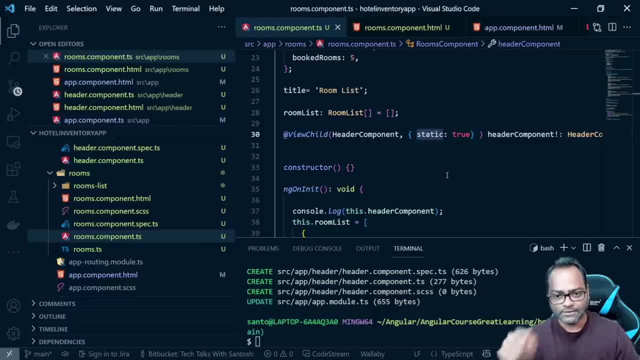 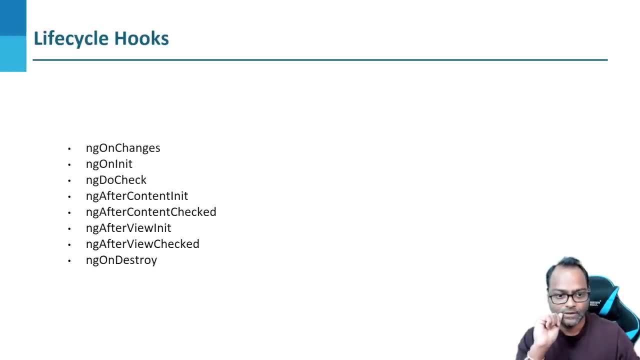 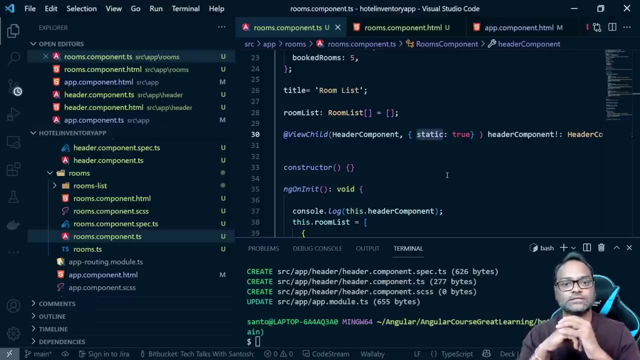 after viewChecked and ngOnDestroyed. As I'm trying to load header component, the same lifecycle of header component will be called as well. Here we are saying static true, which has a very specific purpose. that in case I'm saying this component has this property called with static true. 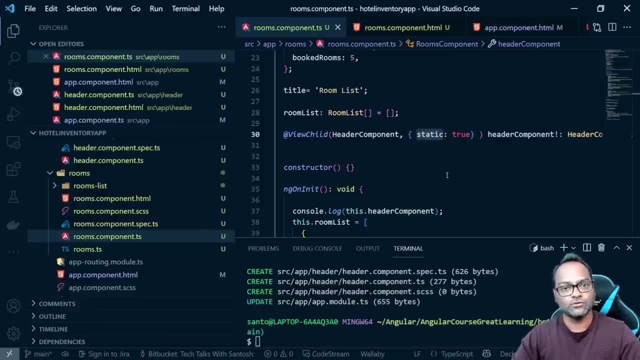 it means this component is actually safe to be used inside onInit of its parent. Why so? I mean why we should make it true and why should we should make it false. This is here where I will talk about little bit. I'll talk a little bit about asynchronous programming. 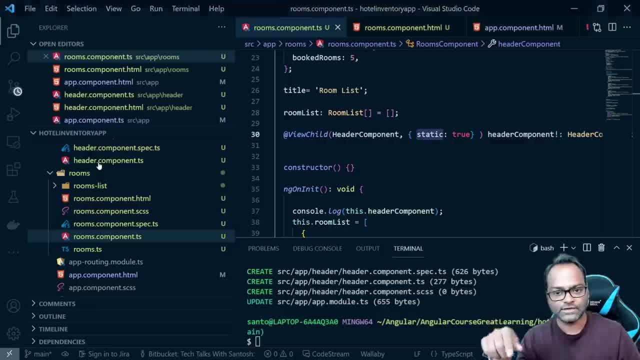 If, let's say, my header component has the same lifecycle look and inside ngOnInit lifecycle look, it has some asynchronous code. what will happen In that case? of course, the execution will be blocked, And it is not. it is not, we won't sorry. 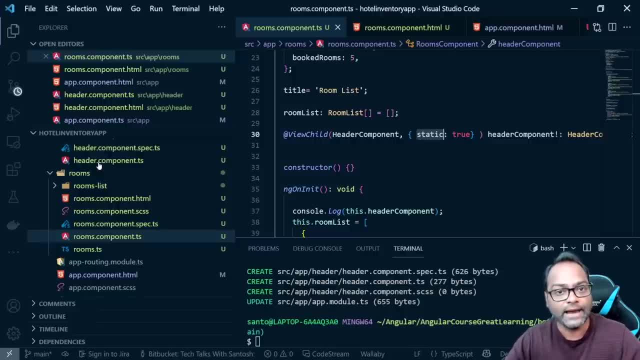 we won't be confident that this particular instance will be available at the ngOnInit of my parent because, of course, I mean at this particular time, header component is still executing its ngOnInit lifecycle. look So it is still not initialized. So whenever you have some component which has 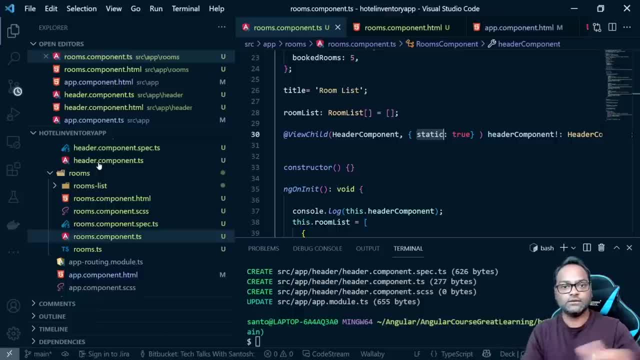 let's say some asynchronous code which may delay something, right, So which may delay creating or executing the ngOnInit lifecycle. look, make it static false. Do we need to do that? No, the answer is no. Static is false by default. that's why. 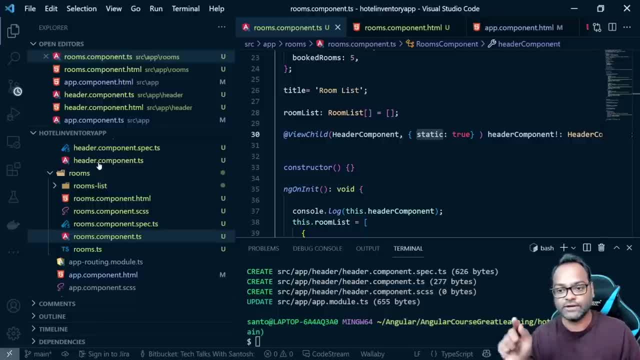 we were not getting that instance at line number 37, when we didn't add it static true property. In this case, header component does not contain any asynchronous code, so it is safe to be used, But still, whenever you are using ViewChild, 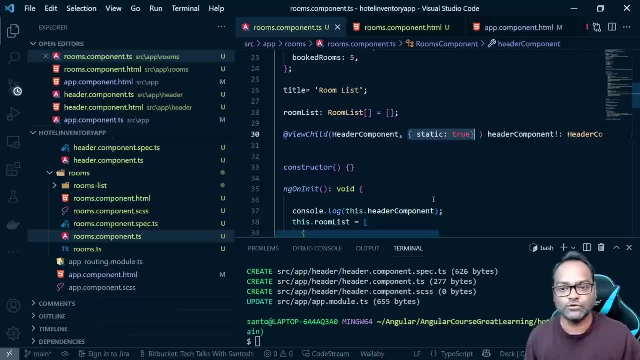 that's why they removed it. So earlier there was a lot of confusion. A lot of developers used to miss this property and they used to try accessing it inside ngOnInit lifecycle, which used to get, which used to cause an error, And developers used to blame the framework. 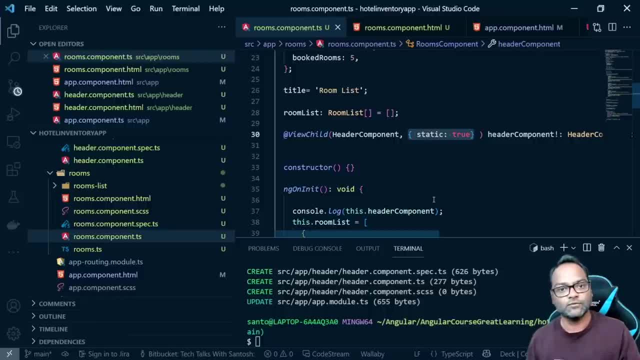 So Angular team decided around Angular 9 that they will remove. make it by default false. So they will make static by default false. So developers don't get any instance inside ngOnInit. In case they are sure that? okay, I am sure that, okay. 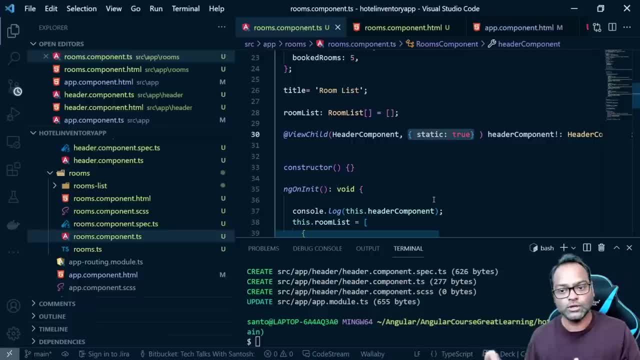 this will not cause any issues. they can make it static, true? So, based on what you are trying to do, use this static property properly. In case you're not sure, just make it, just keep it. just keep it default, So where you don't have to pass anything. 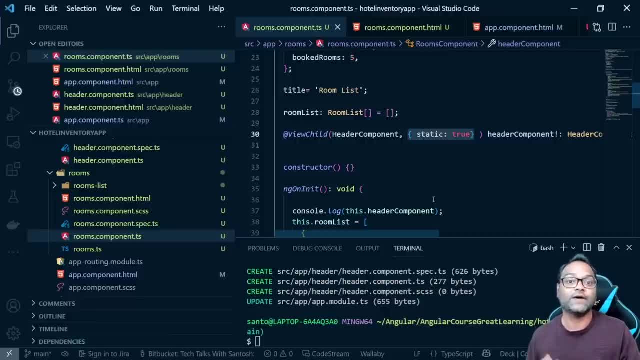 and you are safe to access this instance after ViewOnIt. Now let's come and talk about after ViewOnIt What we did there right, Why it is available in after ViewOnIt. So when we are saying, static is false, of course, 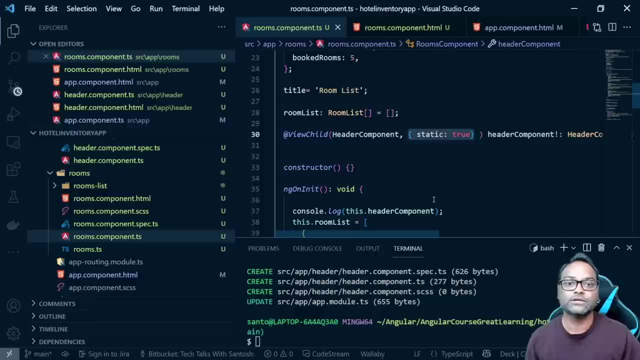 we are saying, okay, this is something which may cause delay and we are not sure that we want to use it inside ngOnInit After ViewOnIt is lifecycle. So ngOnInit is initialization of the component. So component is getting initialized After ViewOnIt is at this particular lifecycle. look. 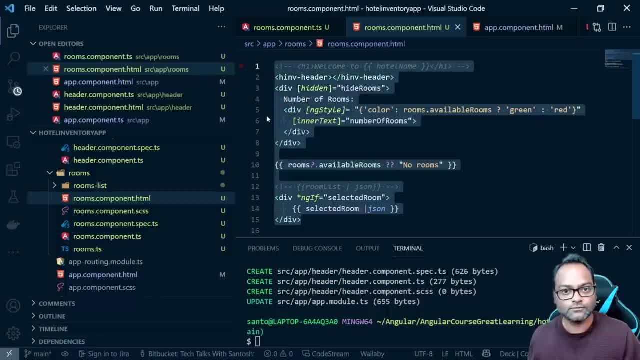 the component is saying all the view, so remember. so the component is saying that whatever view I have, that is also initialized. So if I'm trying to load any other component inside my component, it means that they are also ready. They are initialized as well. 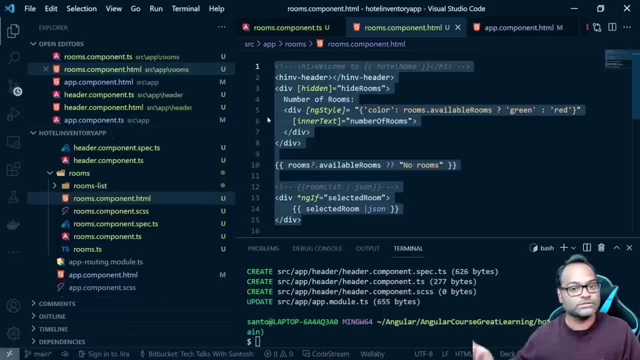 That's why we are saying after ViewOnIt, So after View is totally initialized, after ViewOnIt I mean everything on my template is also initialized- It is safe to use any other component in your template, in your code base, in your TS file. 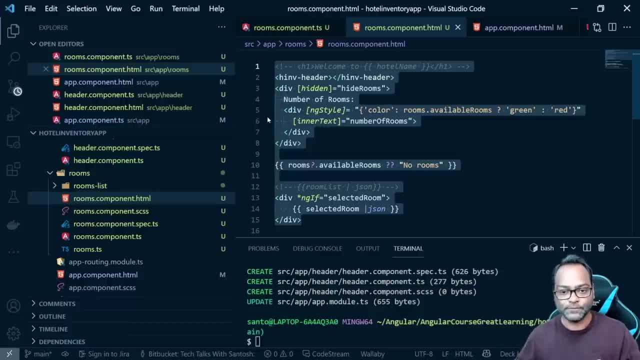 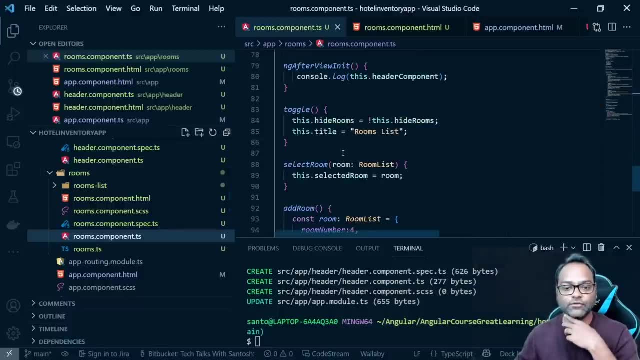 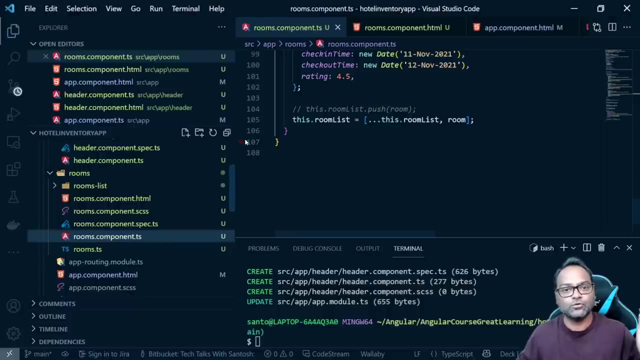 So that's the ngAfterViewOnIt lifecycle. Now the other lifecycle, look, which is related to ngAfterViewOnIt, is known as after View checked. So if you see, here it is known as after View checked. So to go to after View checked, let's do one more thing. 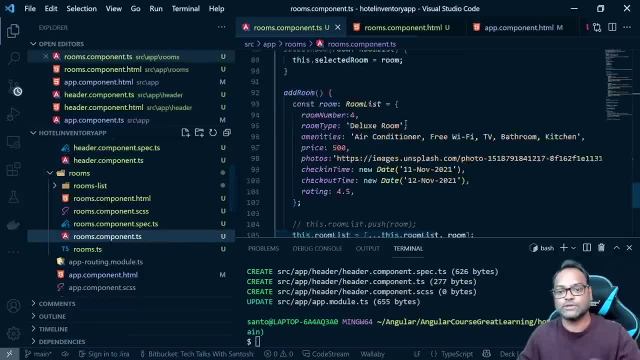 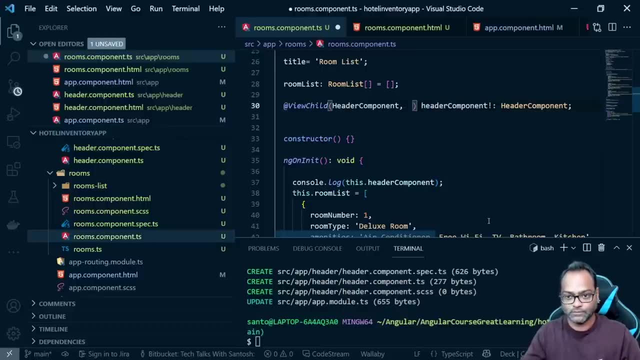 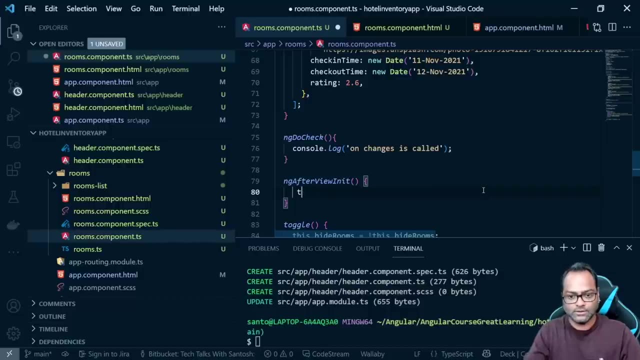 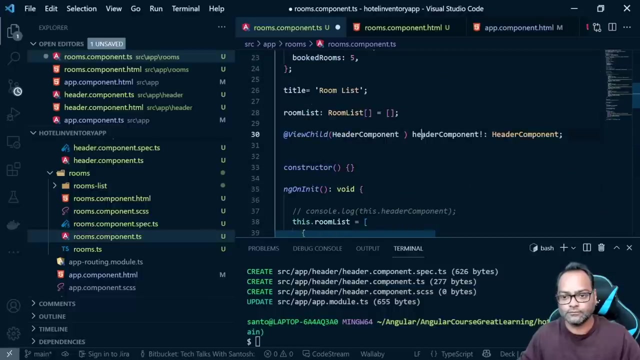 Right now, we have just accessed the instance. What I'm going to do is: I'm going to remove this. I'm going to remove this static property key from here and comment this out, And here let's assign the property title And I'll say: this is OK. so we are saying OK. 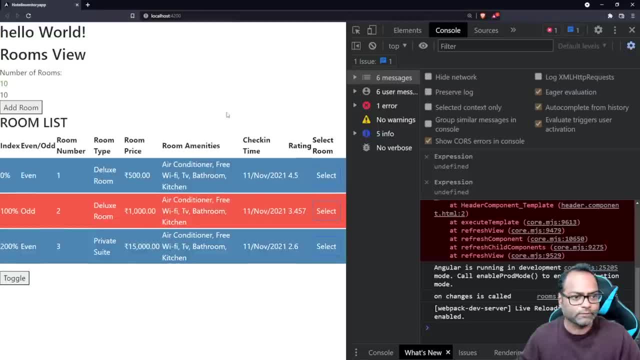 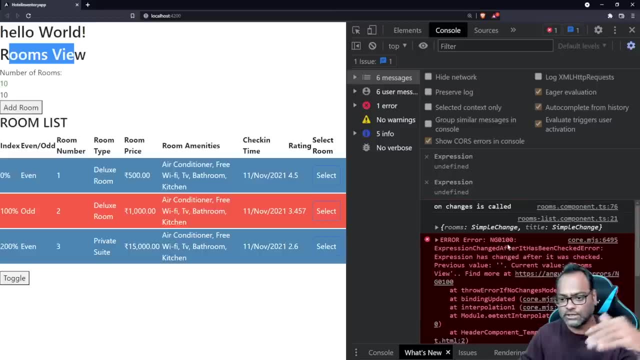 this header component title is RoomsView And you can see the properties available here in RoomsView. But I want to show you one more thing. So here you can see there is an error which says expressions, and changed after it has been checked. 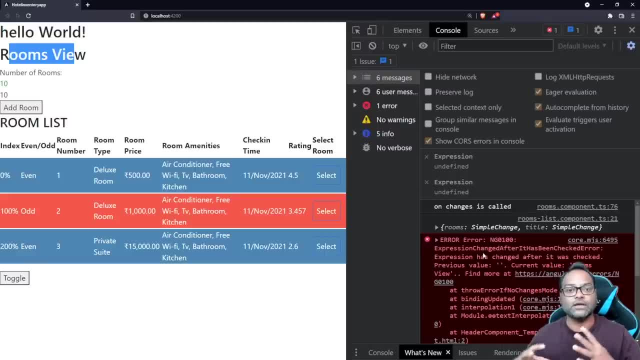 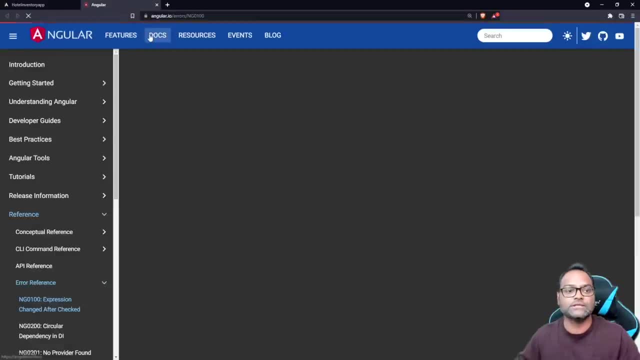 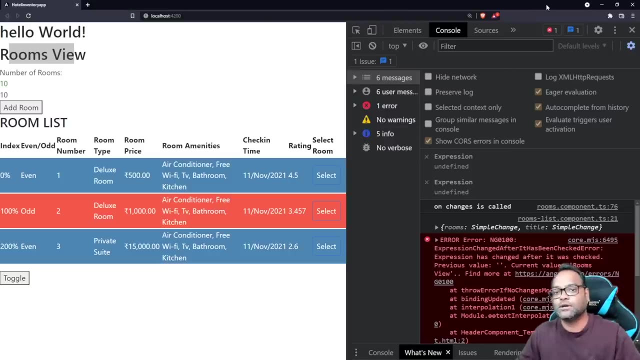 So this is one of the most- what you can say- the most searched error related to Angular, And it has an actually link as well, So you can click on this link and it will tell you more about this error. It has actually a video as well, from the Angular team. 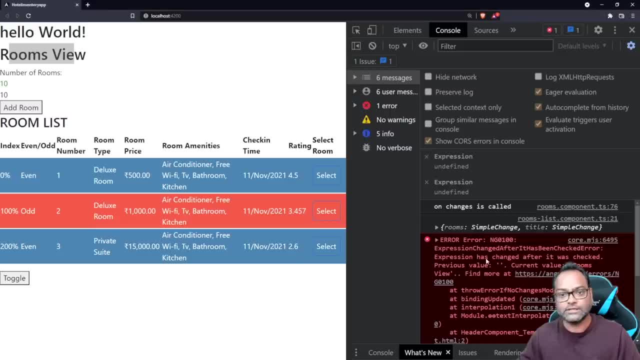 So let me tell you you should not worry about this error. In case you get this error, this is totally fine. if you get this error on your development map, This is the development environment Right now. we are in dev environment. How you can verify if you are in dev environment. 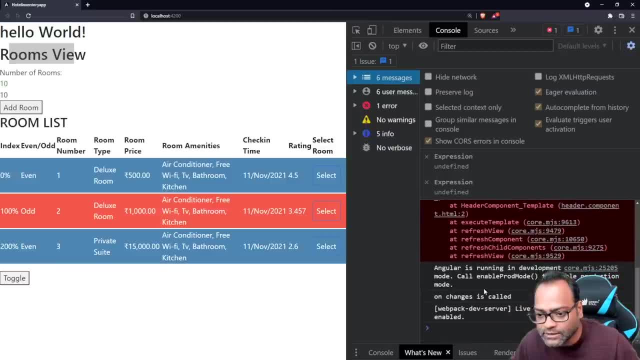 you can just click here six messages and here, So in console you will always see this message: Angular is running in development mode. When you create production build, you run in production build. If you get this error in production build, 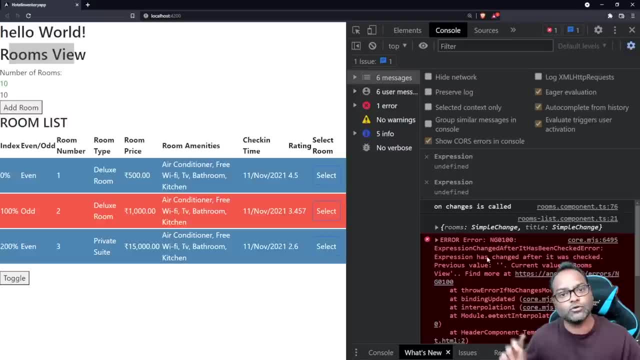 there is definitely something wrong with your code. But if you get this in your development mode, that's totally fine, And let me tell you why. Of course you can go to the link and you can read more about it, But let me just tell you. 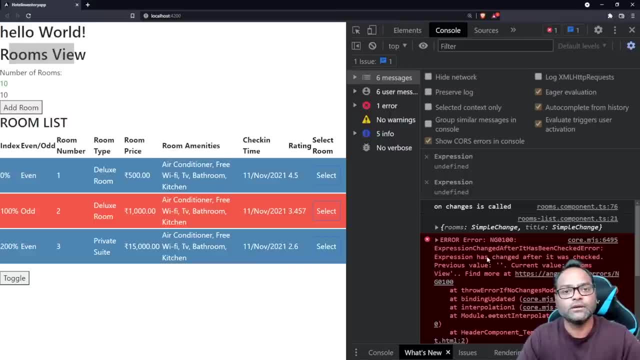 As we are going through this particular topic, in development mode, Angular runs change detection twice, So that's why we get this error. So it says, OK, previous value was blank, Now current value is room's view. So they run it twice. 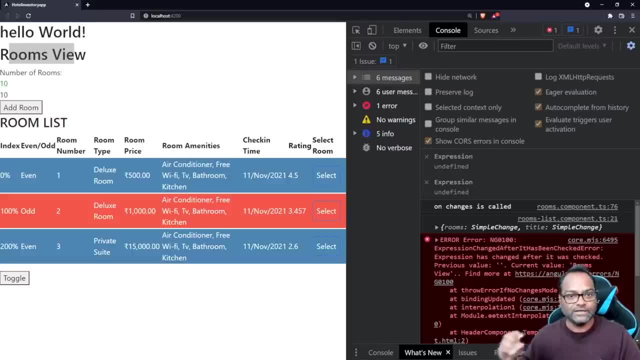 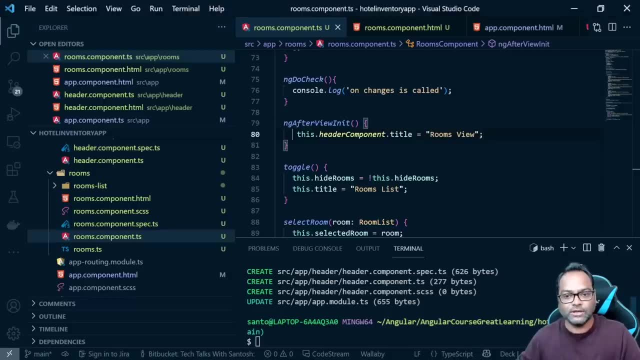 That's the reason we have this error And why they do it, Because it's, of course, development environment. So they need to actually go ahead and recheck if something has changed. So don't worry about it. I mean, it's totally fine. 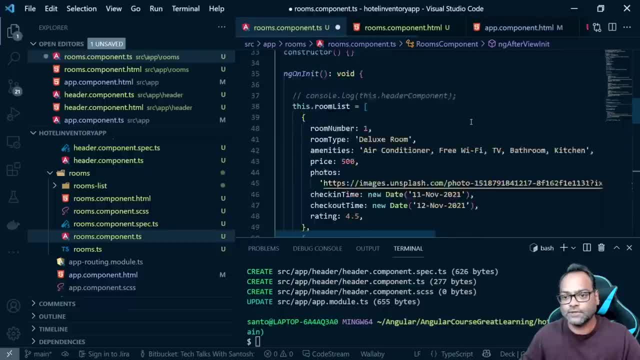 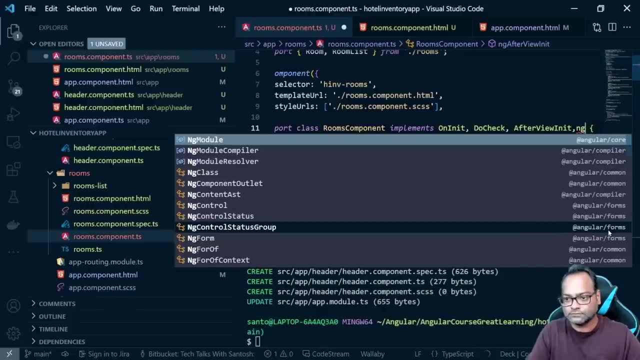 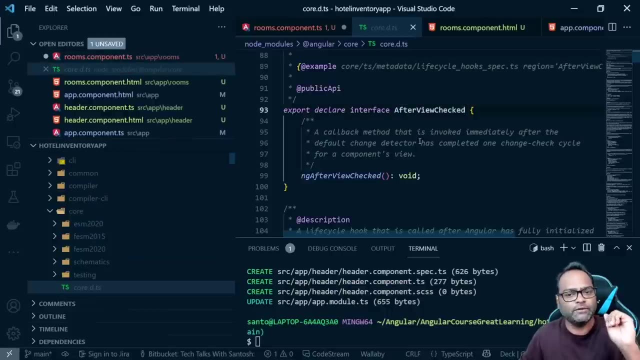 And ng. after Let's view checked So we can actually go to this. after view checked So you can see you probably will never use this particular lifecycle. look, So it says a callback method that is invoked Immediately after the default change. 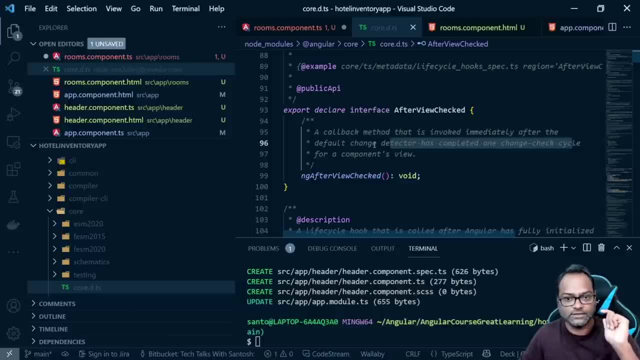 director has completed one change check cycle for a component, But, as we said, we don't need to do this. We will by default- I mean Angular will- run this change detection twice In your development mode. you will get this error. 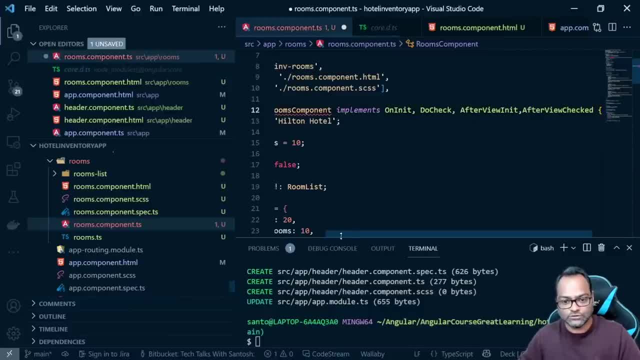 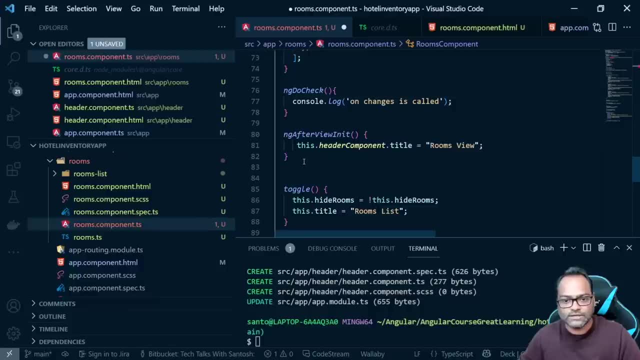 even though we call this in after view checked. So it's like: now let me just talk a little bit about after what we have after view checked lifecycle look. So at this point Angular has already completed one lifecycle check already. So in case you want to, let's say, assign some property here, 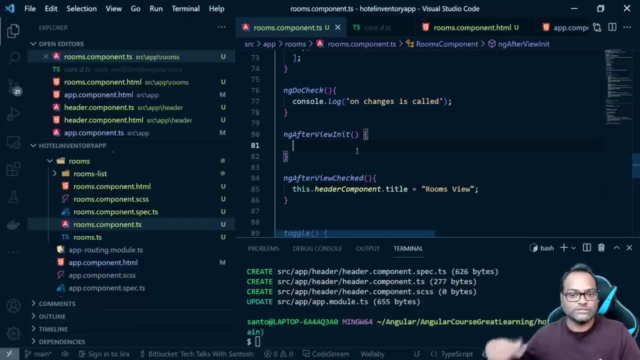 you can actually go ahead and do that here After your change detection has completed. or you want to modify something, you want to modify some values, you want to call some function? you can actually go ahead and do that here. But remember, in dev mode you will still get this error. 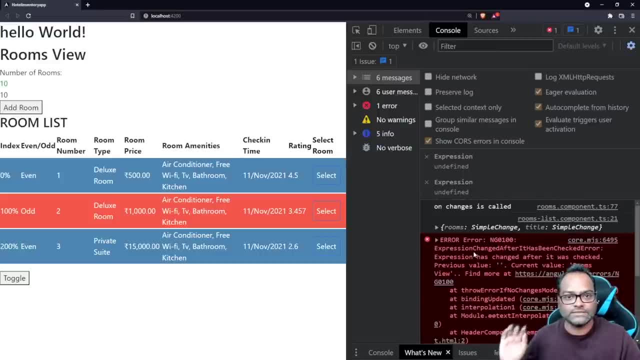 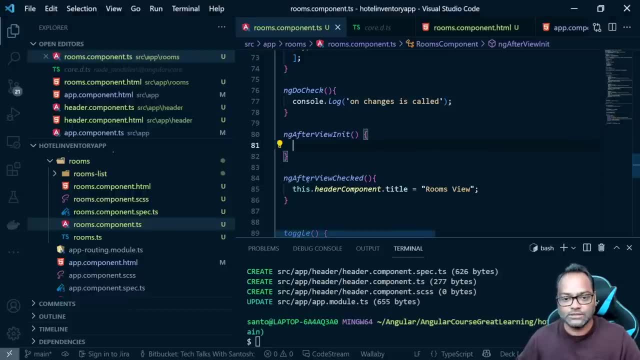 So don't worry about it. This error is okay in case you get in dev mode, But if you are getting it in production mode, that's an issue, Yep. So this is it. So let's go ahead and go ahead and talk about those. 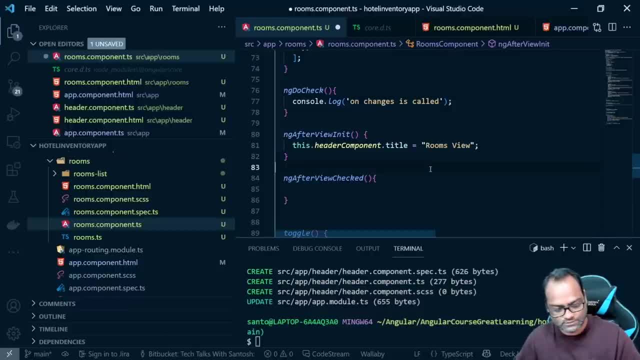 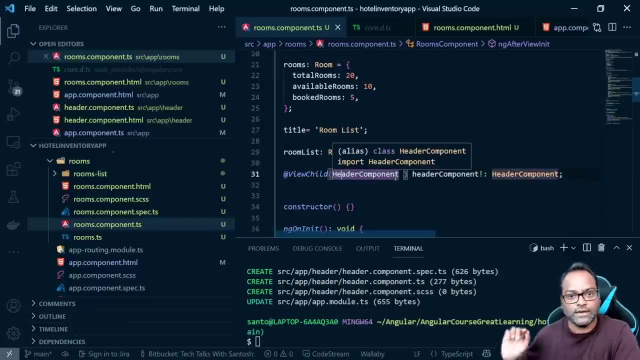 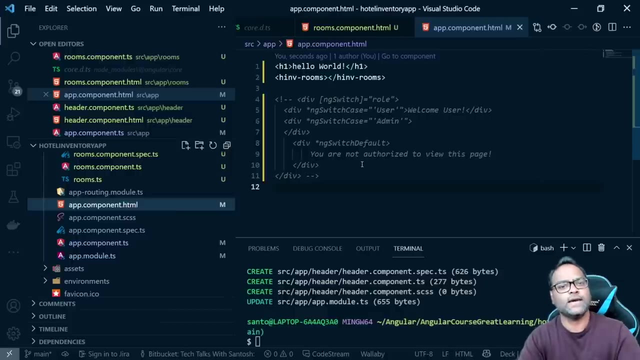 What else we can achieve using ViewChild. Lifecycle looks. I mean, let's do one more thing. How about dynamic components? So let's say, I'll just comment this out Now, I want to render this view as a dynamic component. 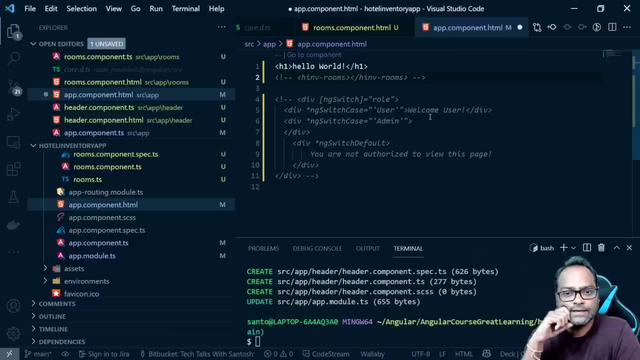 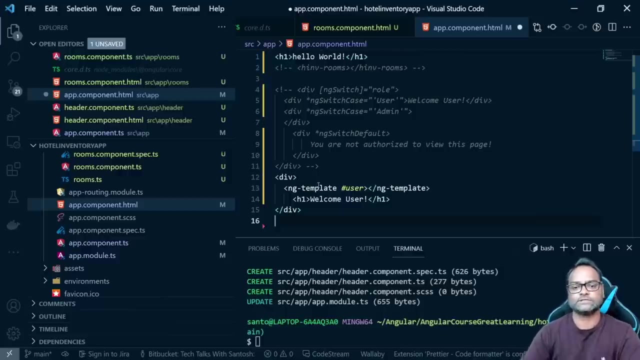 So let's say, I want to render this view as a dynamic component. So let's say, I want to render this view as a dynamic component. So I, my window is in a, so we have this typical. then we have ngTemplate. I will talk about what ngTemplate is. 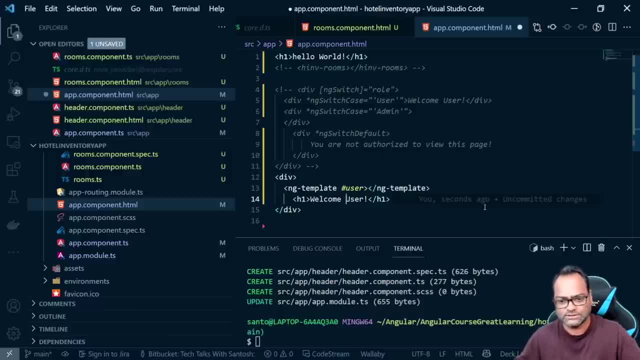 And we have h1tag Welcome User. Let's remove this as well. So we have just an ngTemplate with hashtag user and then ngTemplate. So first let's try to understand what ngTemplate is is. so ng template is kind of like a tag to understand it in. uh, like easy words. so ng. 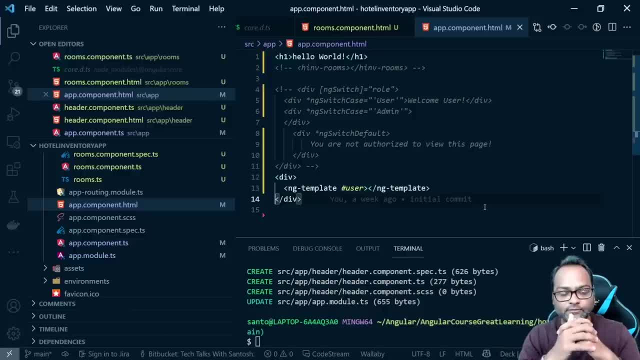 template is a tag which will be uh, which will never render anything, so ng template itself won't render anything, so it's like it is not visible. i mean so, but it can help us to render some other template. so what's some other template can be? it can be another component, so let's try that out. 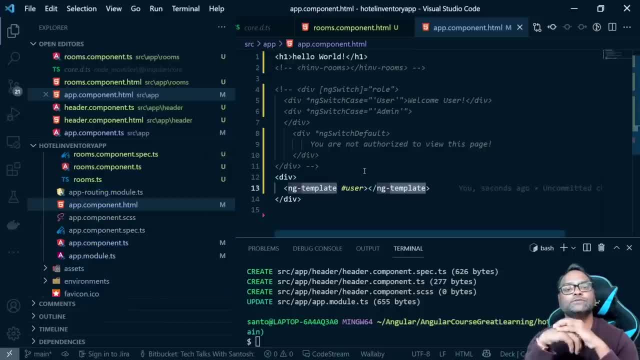 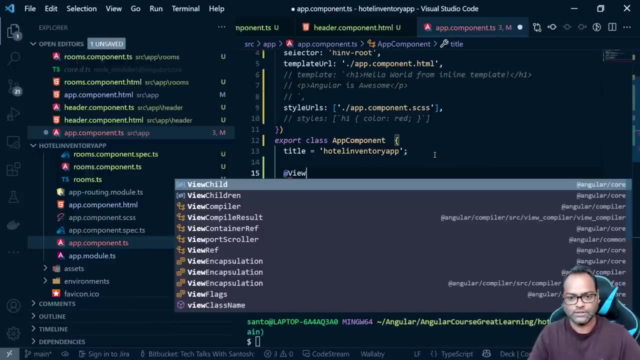 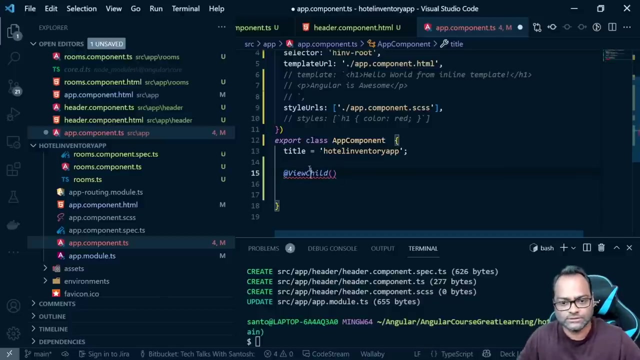 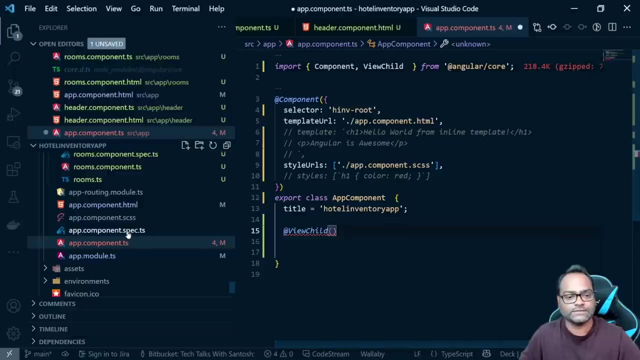 here. what we are going to do is we are going to dynamically load the rooms component using view child. so let's do that. so i'll say, okay, this is view child. and then i need the access. so let's view child and close this. um. now, after this, i need the access to this particular ng template tag. so this hashtag. 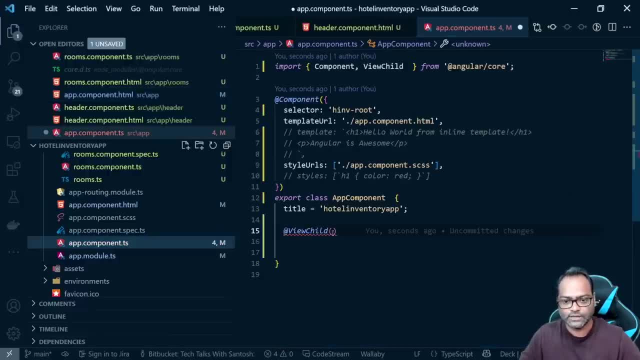 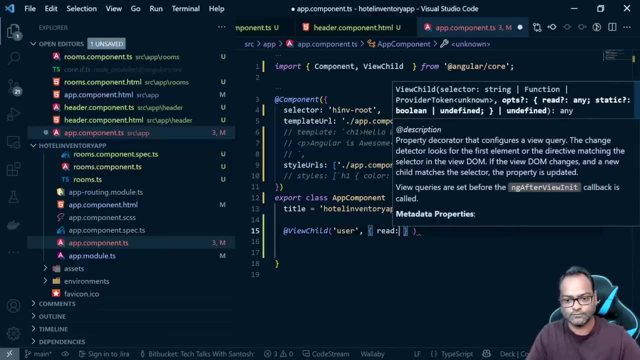 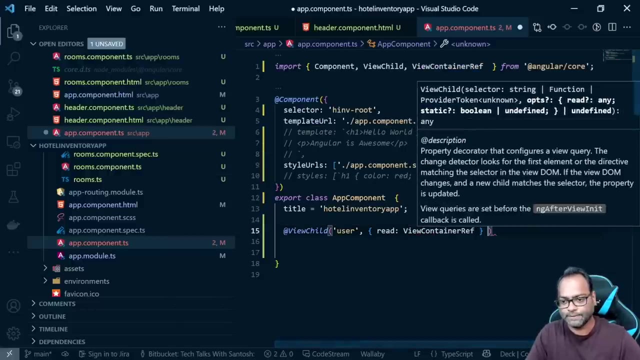 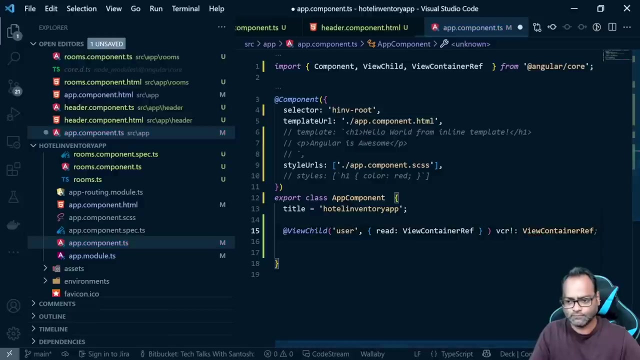 user has some specifics. i'll just talk about it so we can use this here. and then we can use one property called read and which we can pass view container web. i'll call it as vcr view container, which is type of view container web. it is going to give me some reference by the name, if you can guess. so it's saying: okay, i get it will. 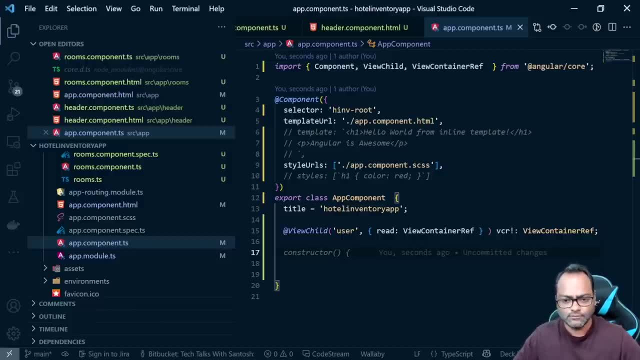 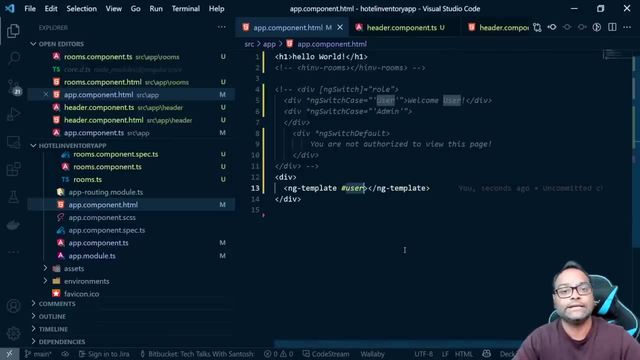 give me some reference to what. now let's talk about this user. so here, this hashtag user is something known as template reference. once you define something with hash on any html tag, you can access that tag. you can access that tag. so you can access that tag inside your ts file using view child. it's not only with ng template. i. 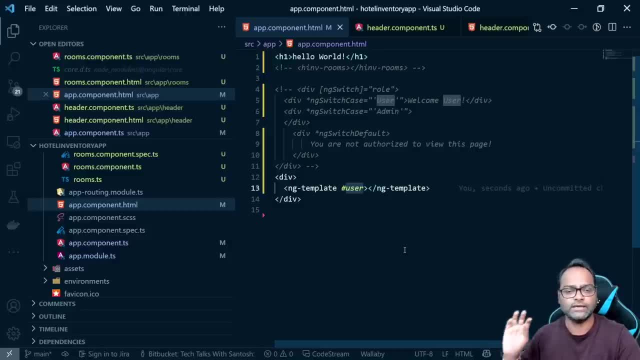 can access any html tag. i can even access div. i can access even input element. we'll talk about it, i'll. we'll see an example right to, just to be sure that how it works. so here we are saying: give me the reference to this user tag, right, and this view container. 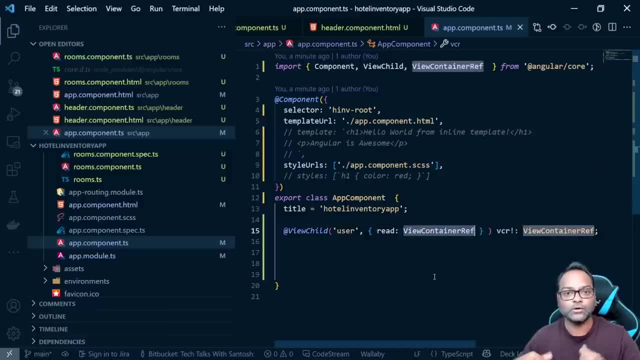 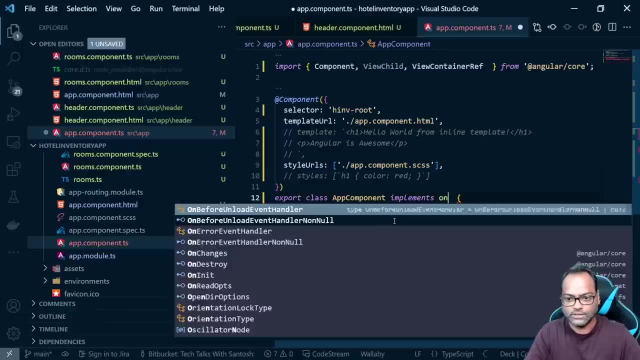 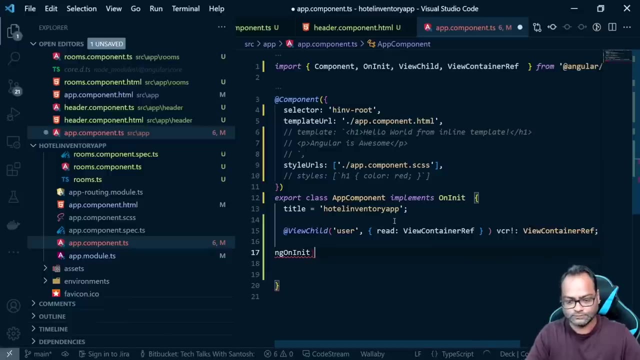 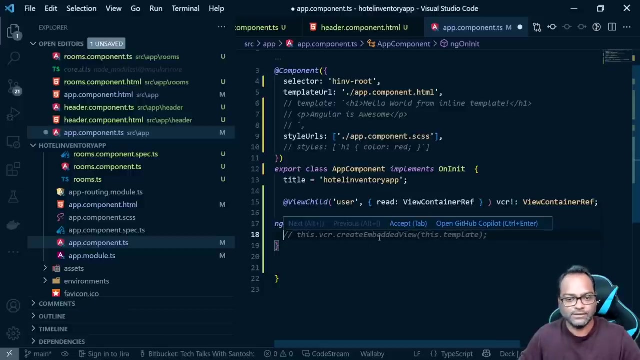 ref will actually help us to dynamically load a component. let's do that. so here i'm going to first say it implements on init, and here i'll say this ng on in it, and uh, okay, so i'm getting some uh hint because i'm using some service from github. 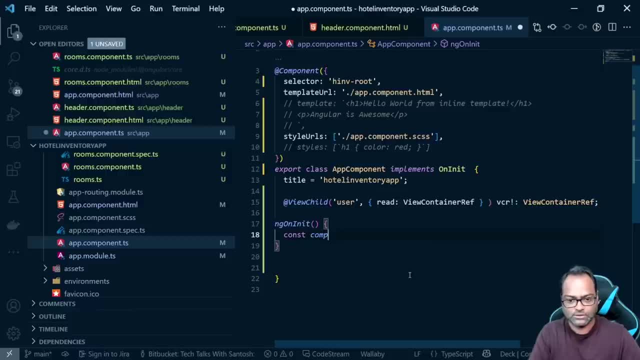 so i'll write this code, so i'll second const component as you want to. let's uh, assign some value as well. component ref is equals to. i can say this: dot, vcr, dot. so there is a method. okay, so you can use this: dot view container, ref. dot create component, and then you can pass. 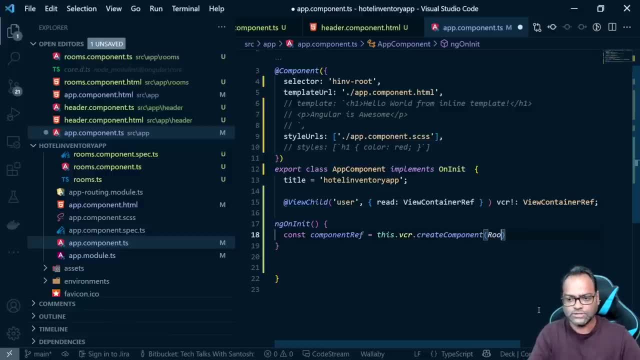 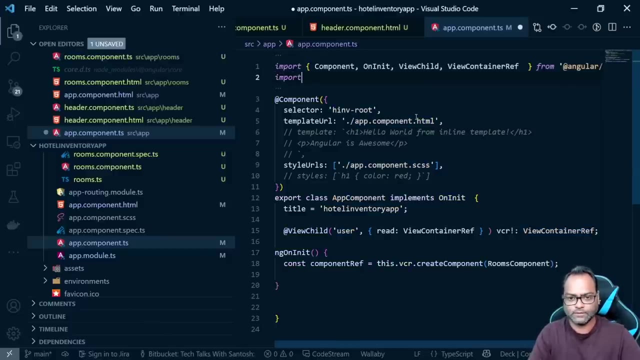 any component here directly. so i'll say, okay, i actually i wanted to do: uh is load rooms component and let's import okay. so now, so it has rooms, slash rooms, dot component, so this is the file and then we need rooms component here. so at this point of time, uh, 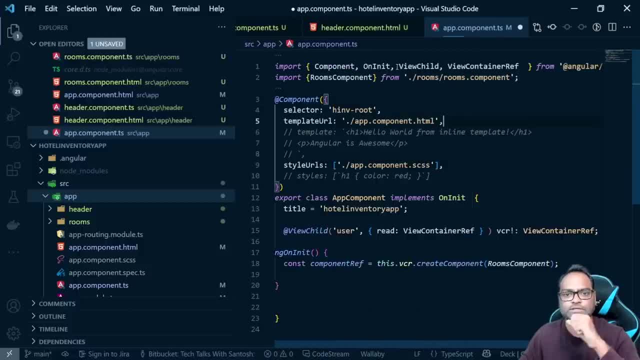 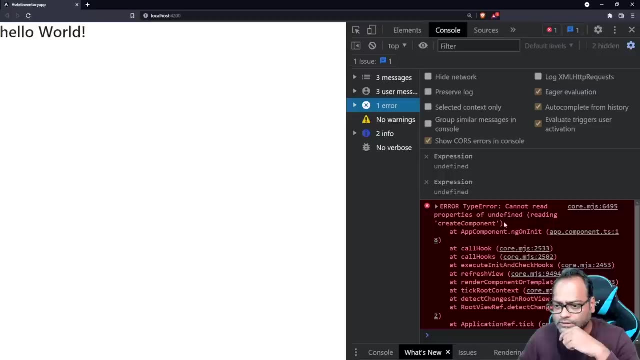 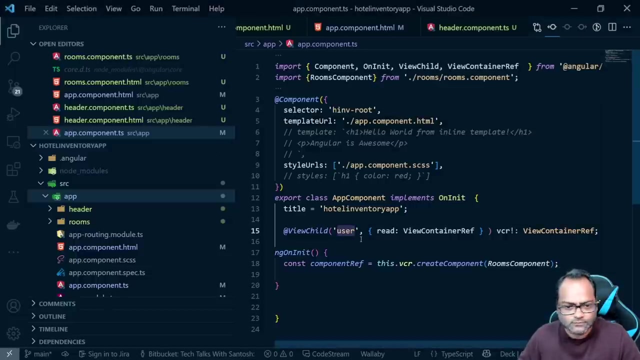 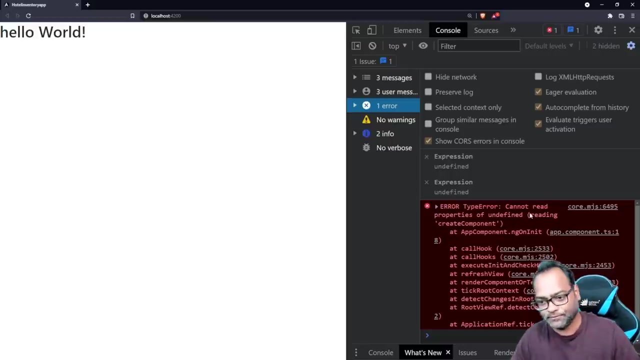 you will see your component will be loaded, so let's save this and see if our code is compiled. yes, it is. let's go to html. and cannot create properties of undefined. okay, sorry so, we just uh. sorry so we just learned that whenever we use view child, the 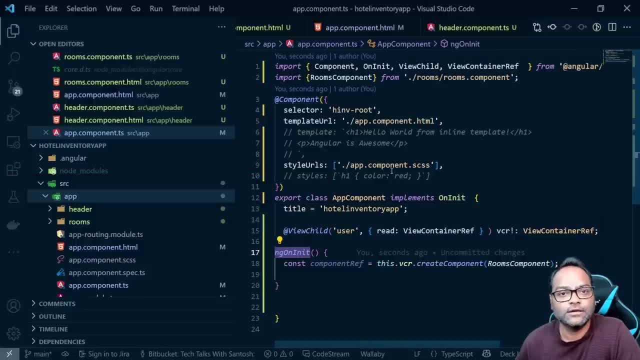 static property is false. so what we need to do is here i'll use val ah and we'll have our atta and let's refer back to our default view question. so after we Manager tab quite a bit, static properties are thrown on the page right now. so you come in and close windows, uh, and 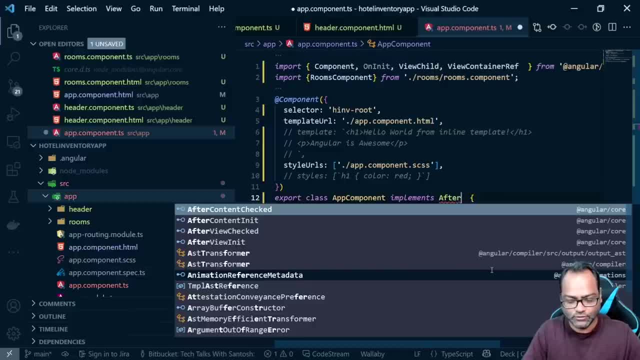 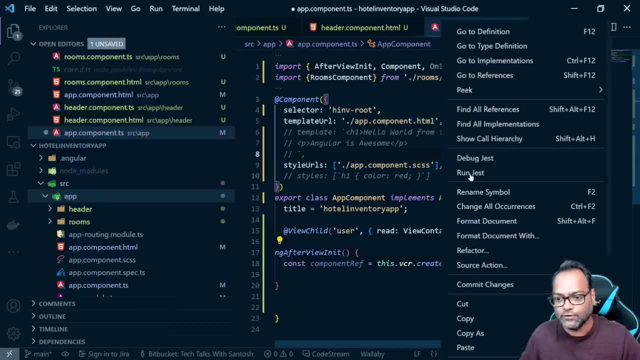 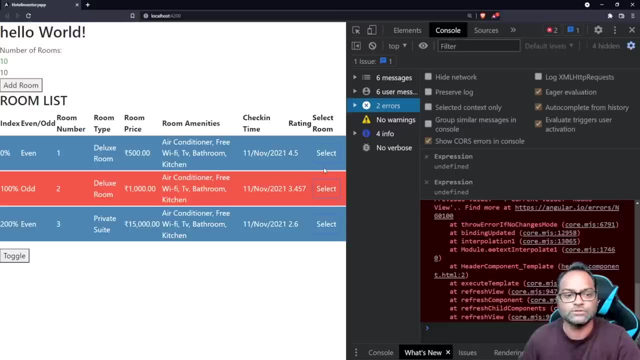 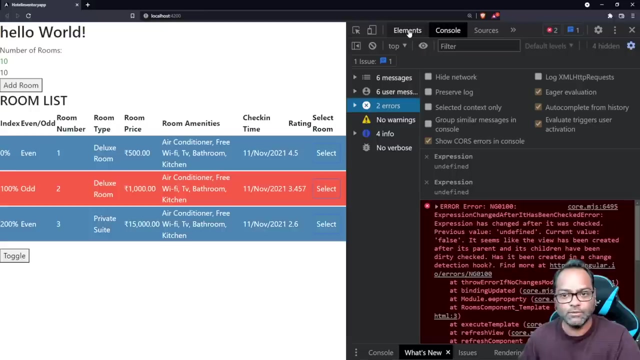 you may need to, i need to use after unit, and here we can access this ng after unit, and now we will get the instance of the tag and it should work now. so let's uh see, let's go to the browser and here it is, so you have your uh view which is loaded, which is loaded dynamically, you remember. 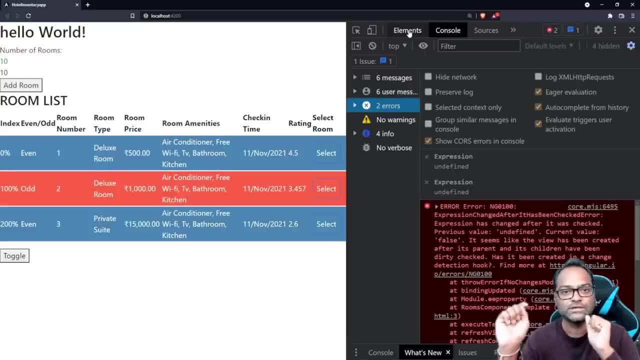 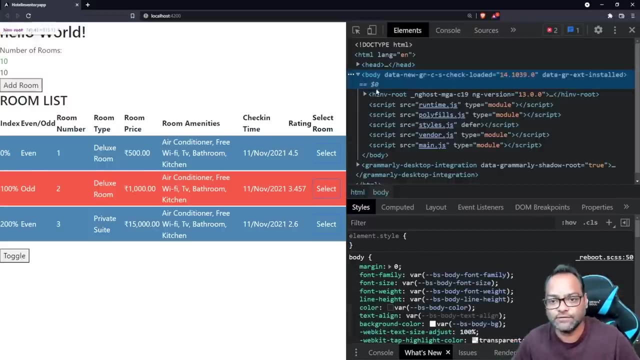 you- uh, you didn't specify the rooms, uh, component inside your template. inside your template, you just have an ng template and you just gave a reference, a template reference, and then we loaded that component dynamically from our typescript file. so this is what you can achieve. you can just let's. 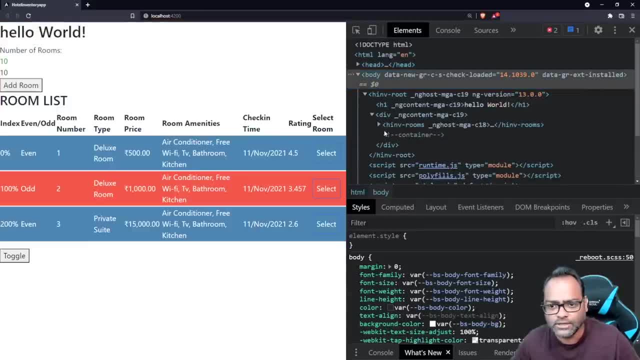 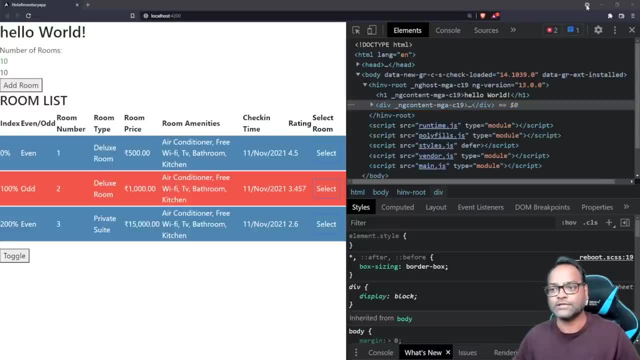 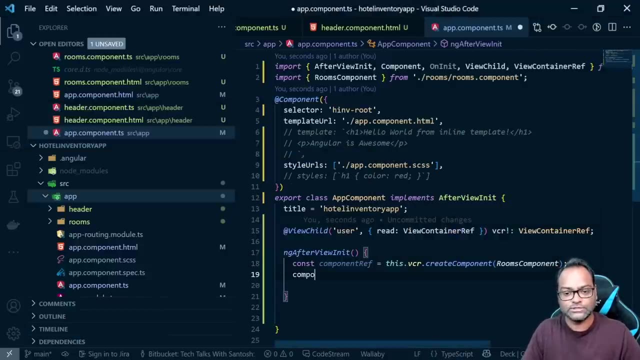 see the uh html dom. here you have hinv rooms which is loaded inside this particular div. and this is it. this is how you can actually load a component dynamically: just a single line of code and, in case you want to actually modify some properties, using component ref. so i can. 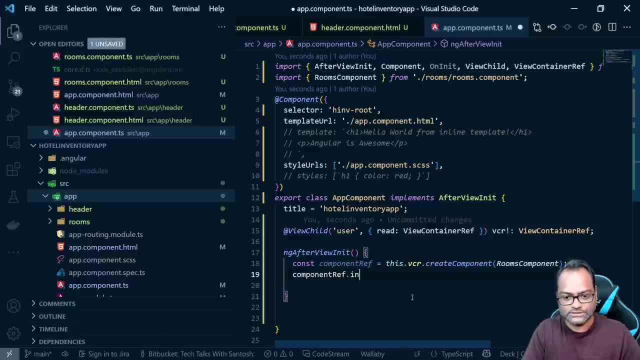 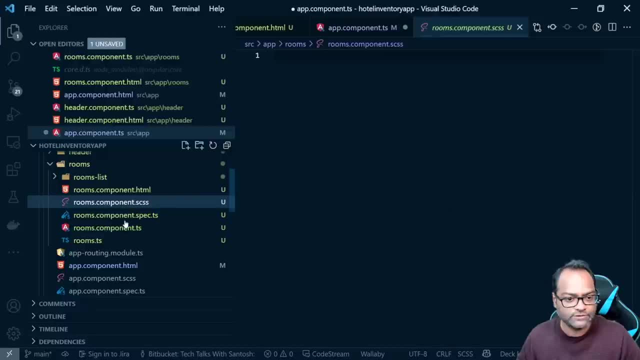 just do component rev and i can do instance dot and you can access any property. so let's try to access any of the property which we have available here and i'll say number of rooms. it is 10, right, so let's try to change it. it is getting used somewhere, yeah, here. so i'll say this: 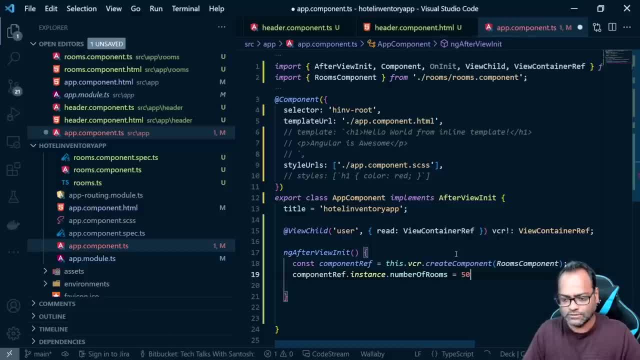 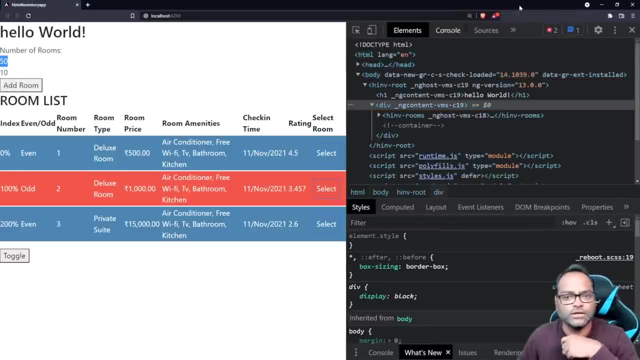 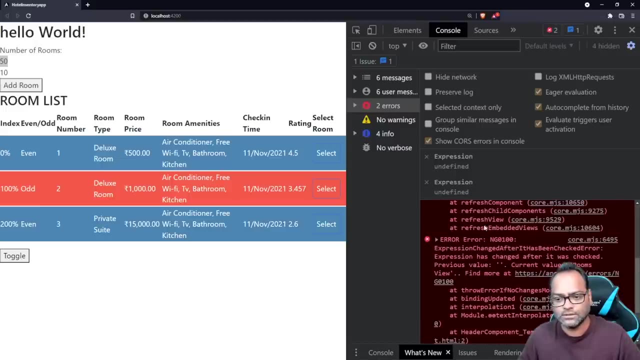 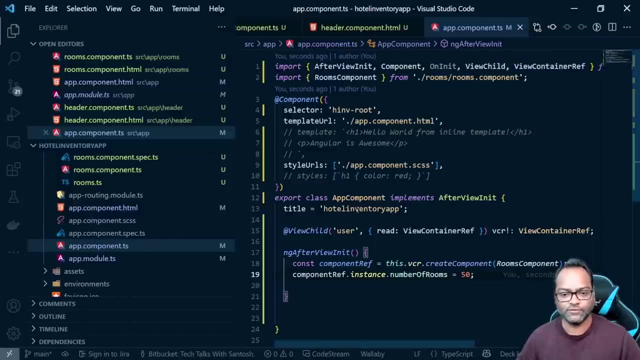 number of rooms, as it goes to 50.. let's, let's run it and see the output here, and you have 50 here. so then you have actually loaded a component dynamically. you changed a property as well, and this is what we achieved using viewchild, and we also learned about template ref. so let's try, uh, to actually access. 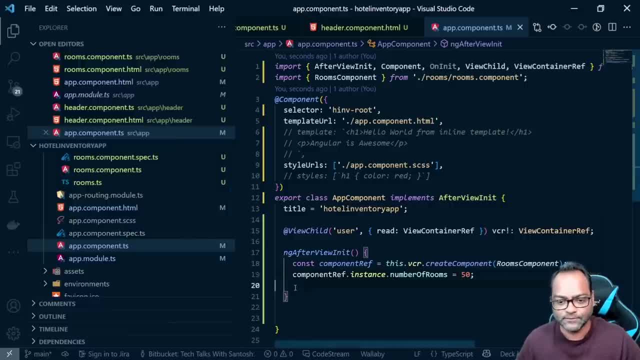 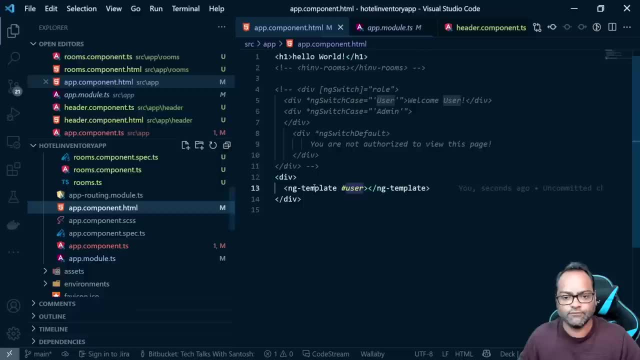 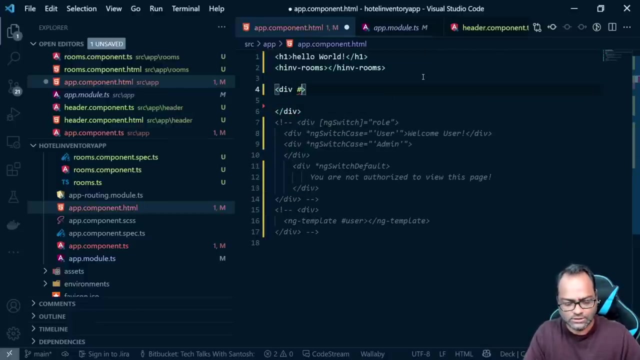 a div element using template reference. let's see how we can do that. i'll just comment this out and we'll keep the code same here. let's comment, uncomment this and here i'll create a div and i'll say hash um any property name. let's say name. so we have this div with hashtag name. 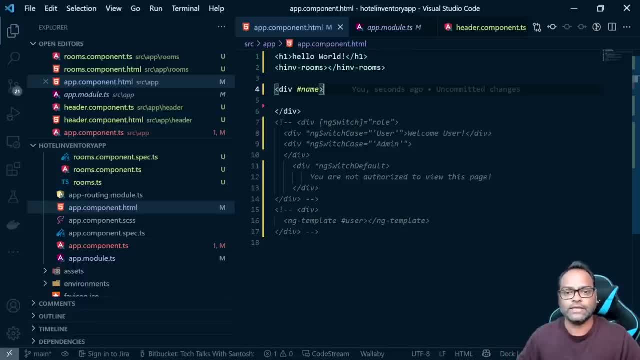 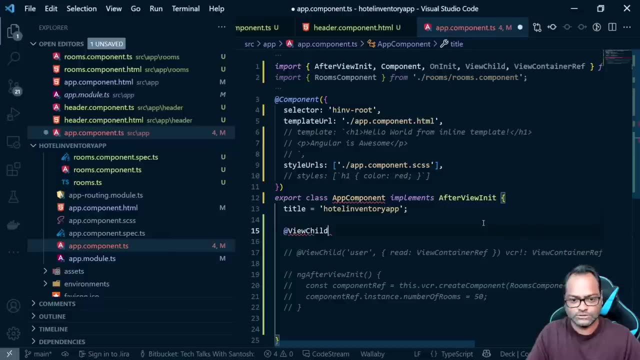 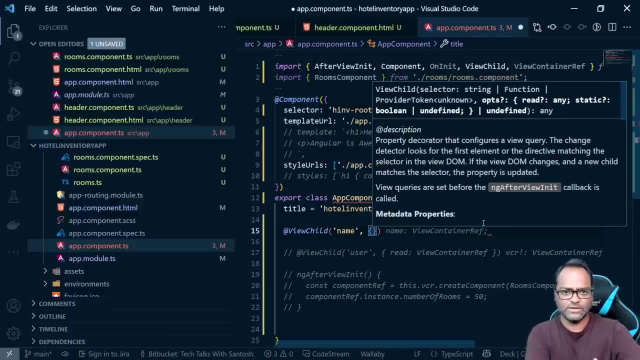 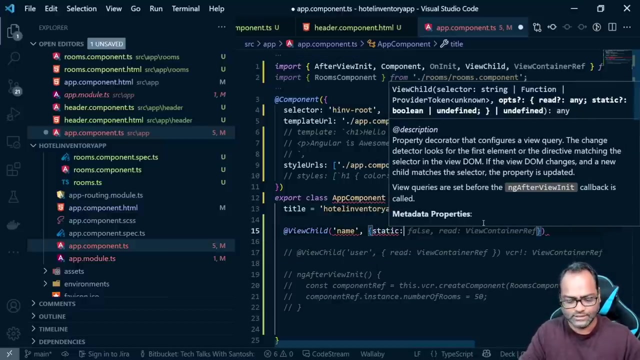 this name is actually template reference. now i can access this inside my component using a view child. i'll say view child, give the name. and now, as i'm sure that, okay, this div is actually available inside my template and it doesn't contain any code which will delay or cause any issue, i'll say, okay, this is static. 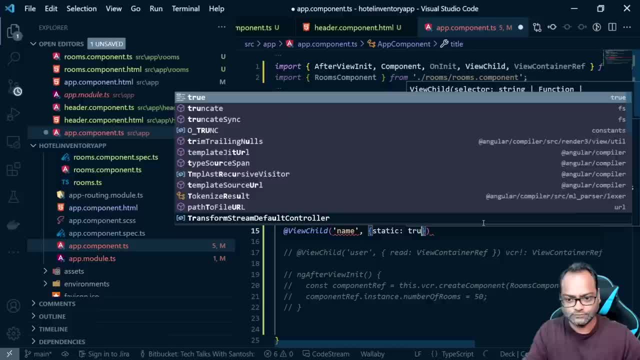 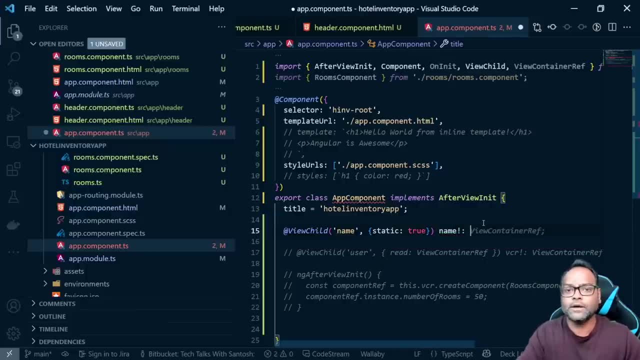 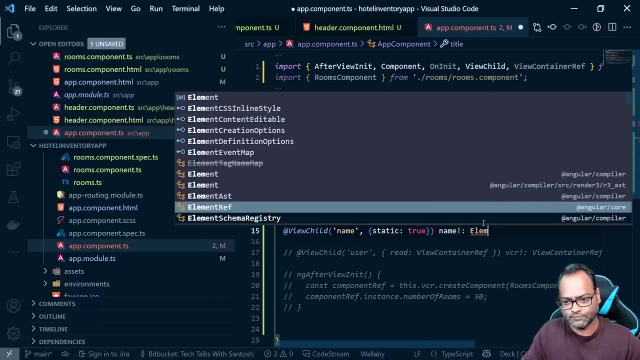 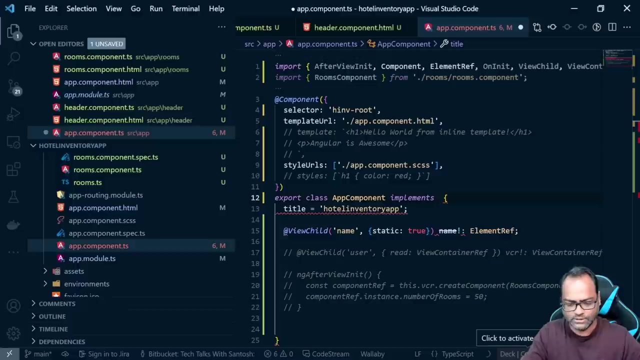 true, right. so i'll say this is name and you can. of course you need to give some type. so you can give a type called element ref, because it's an html element, and now you comment and use on init and let's see it and you're in it, and then i can say this: dot name. 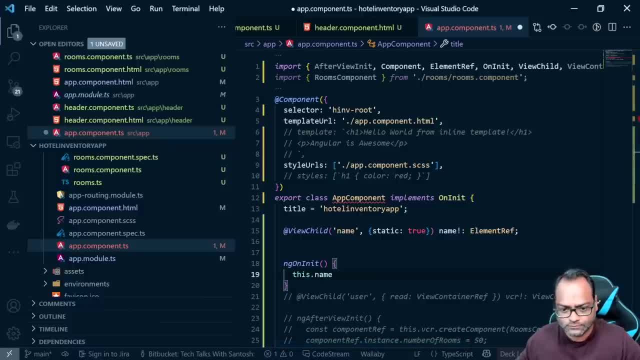 dot in a let's try to access any property. okay, somehow intelligence is not working in, but it should go. give me native element. let's see, let's do consoleorg. so first let's see what this dot name gives us. it should give us an element. so 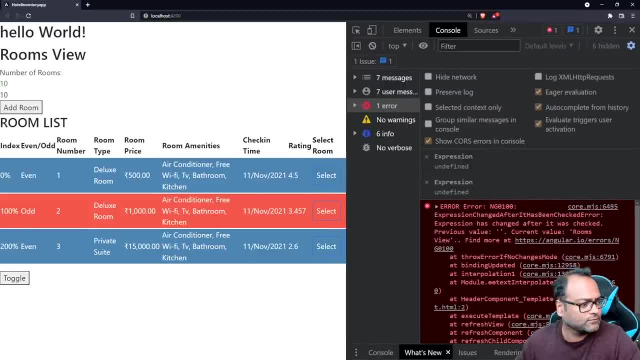 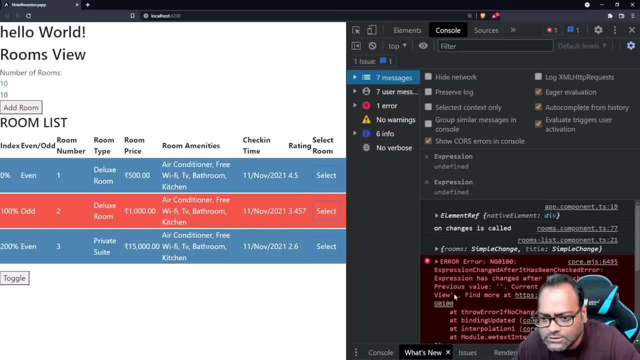 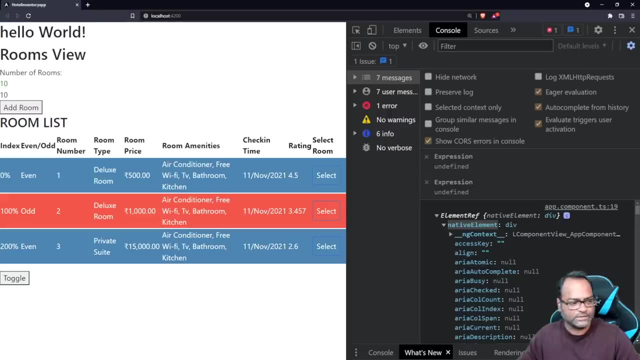 let's see if it is compiled. okay, so let's see if it is compiled. yes, it is compiled. and let's see, here we have native element, ref and yep, so native element is the property which we should be trying to access. so we have, uh, this dot, native, dot, native element, and then 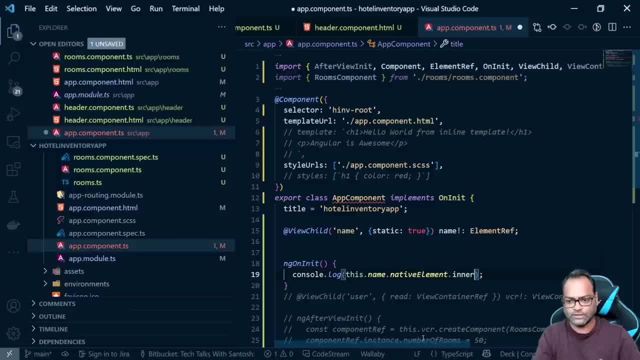 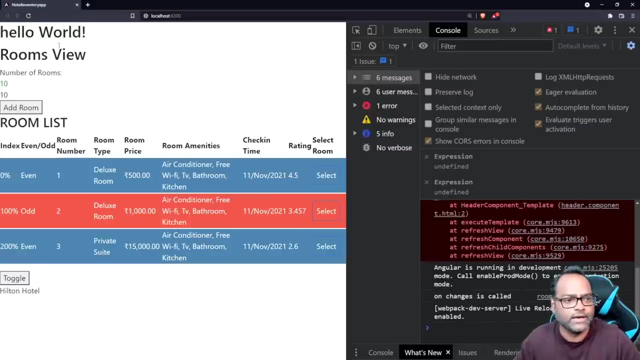 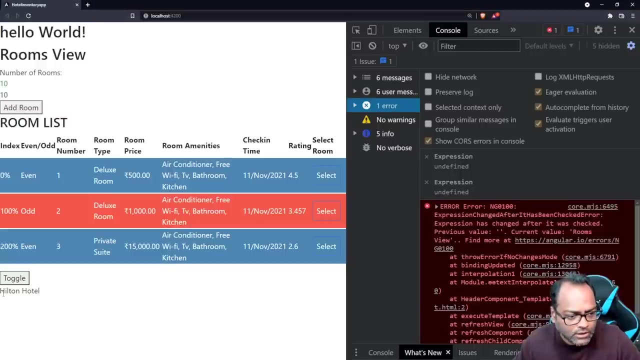 you can access any property. for example, i want to set in a text i can say equals to uh, built-in hotels, and then i will just remove this: uh consolelog. now let's see, and we have hello world. is there any issue? you can, uh, you can see it here. so you have built-in hotel. 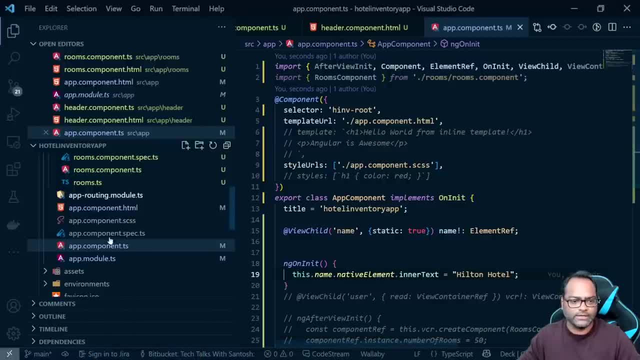 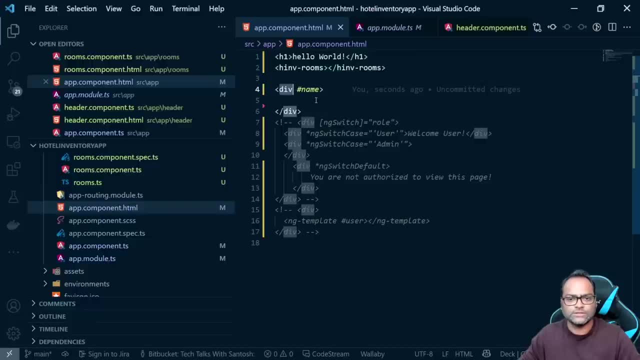 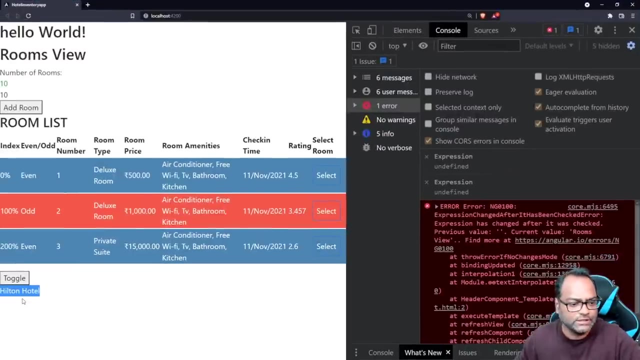 available here. let's put an h1 tag so it's visible right now it is not, or it is, it's okay, right. so we add: uh, even, uh, it's available. so, yeah, that's what we wanted to verify. so we have this little downloadable here and what we did, we 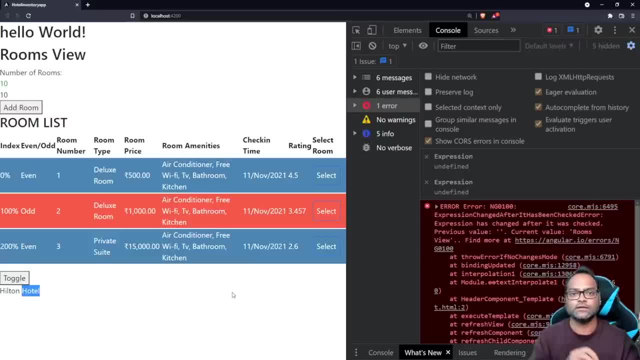 accessed an element. remember so earlier it was like: uh, what, what, what we have done so far using which right? so first we uh, we uh actually accessed and component instance using blue child. that was our header component, um element table which we had um header component right. so we actually accessed header component or created a new instance using typescript. 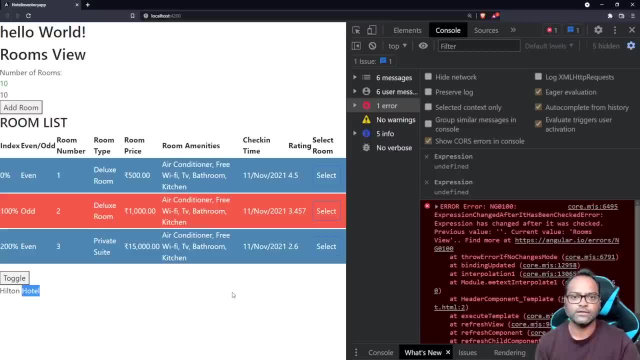 using your ts file. we used view child for that, then loaded it. then we spoke about static property what it does. then we saw in second example where we used view container ref. view container ref to dynamically load a component. that was the second example. third example: what we did is: 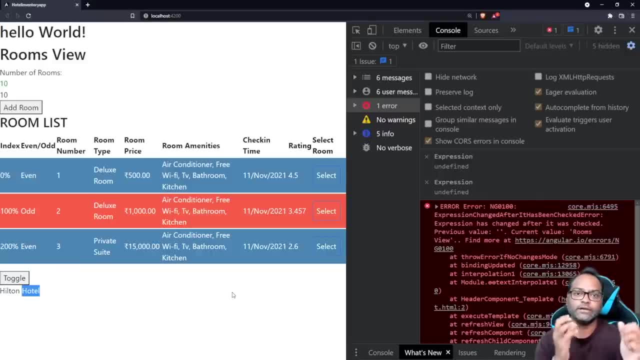 we accessed an html element. we tried, we got the access of that html element using using template reference and then we assigned some value to that particular html element by using, of course, the native property right. so we used, instance, dot, whatever property, not we used native. what was that property name? 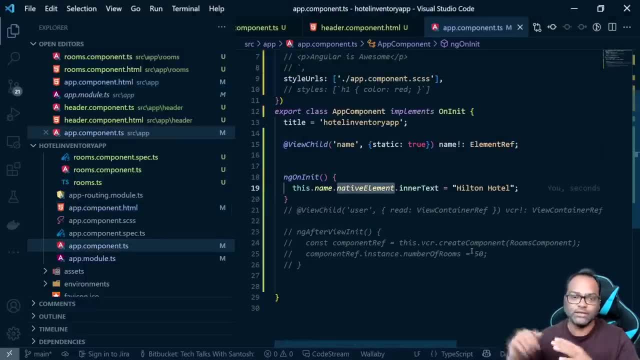 yeah, so we use native element property dot, the property which exists on html element. so here we know, okay, div has something called inner text and we use that property to bind it. so these are three examples which we have seen using viewchild and we also saw that, okay, the instances will be available in case we- you, we- are using static as. 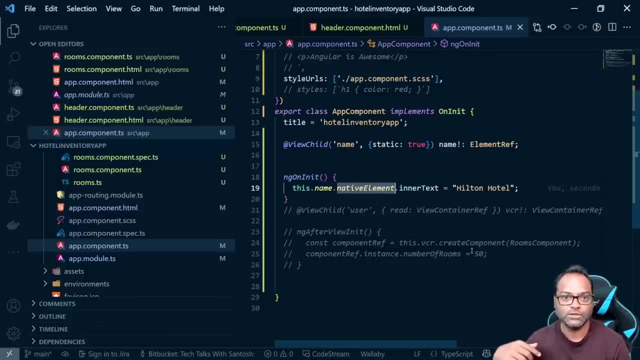 false in after view: init lifecycle: look so most of the time after unit life cycle hook is uh, good for anything which you want to do after your view is initialized and uh, if you checked is it's optional. i mean you will probably there. there, there will be hardly. 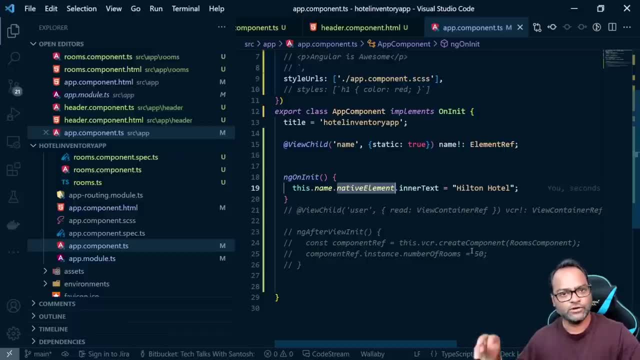 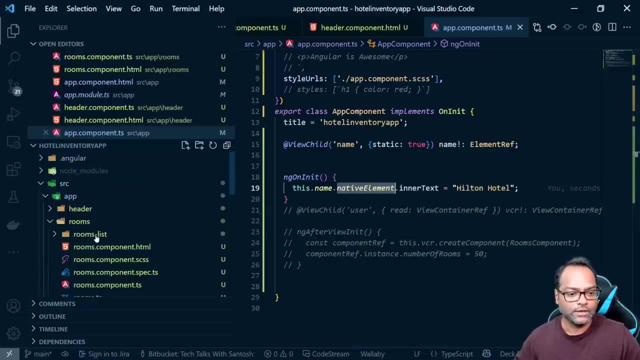 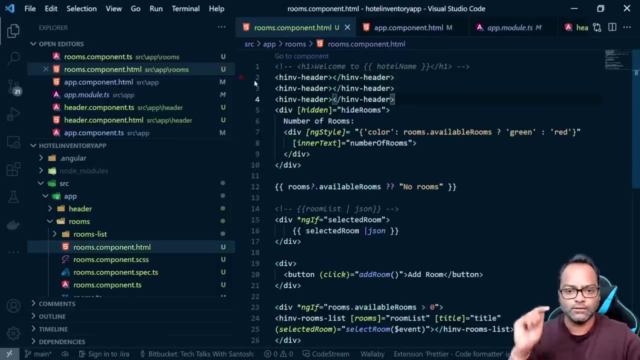 some instances where you will find it useful, but you can do everything which you want to do after view is initialized inside ng, after view init lifecycle. look now, let's see one more example. i'll do one thing, so i what i'm doing is i'm having multiple instances of this header component. 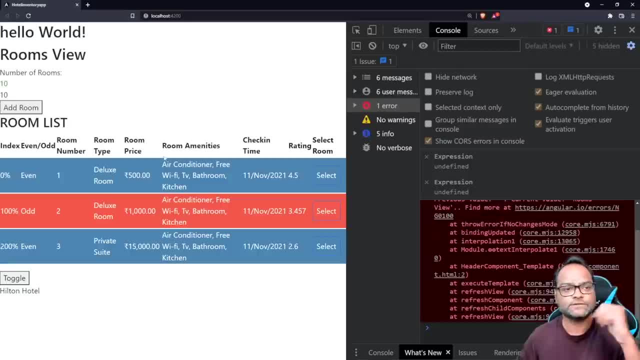 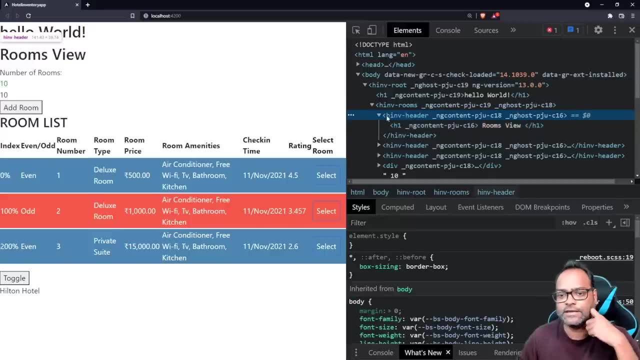 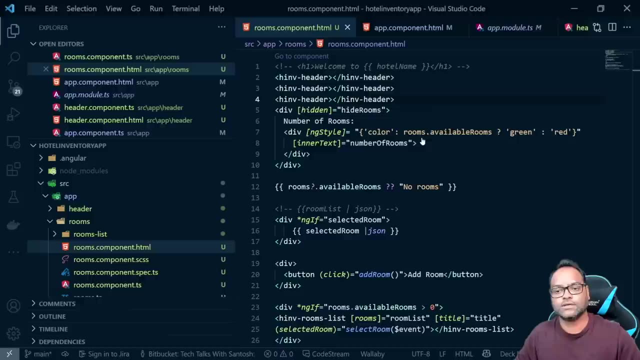 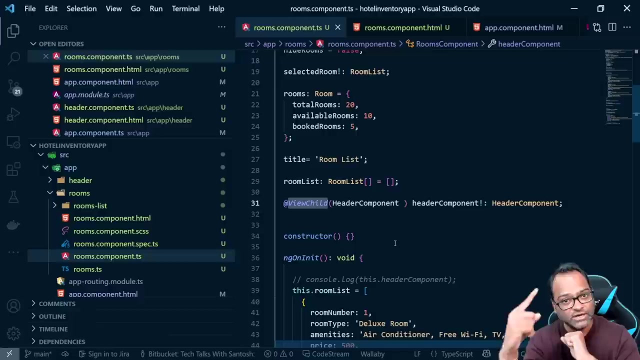 inside my rooms list let's see how it behaves. so we still have single here. we still have only one instance which is available and which has this rooms view property rest doesn't. so here let's try to understand this: view child property will always access the first. 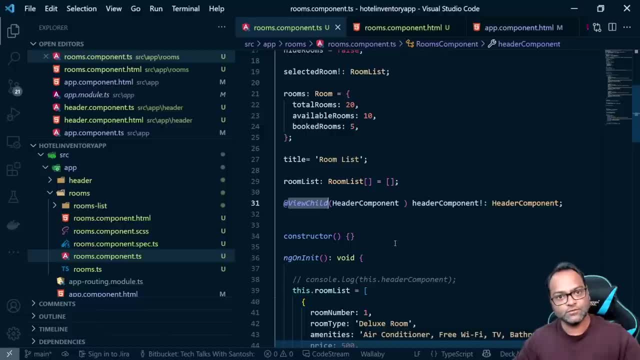 instance, which is available on your template. in case you want to access all the elements which is available, uh, on your component of type header component, you need to use view children. so name itself tells you what we are trying to achieve, right? so view child, in case i have. 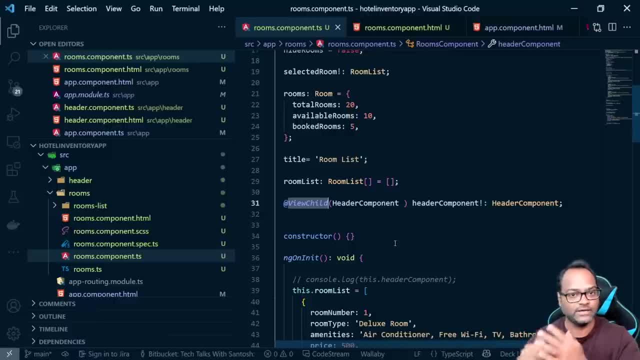 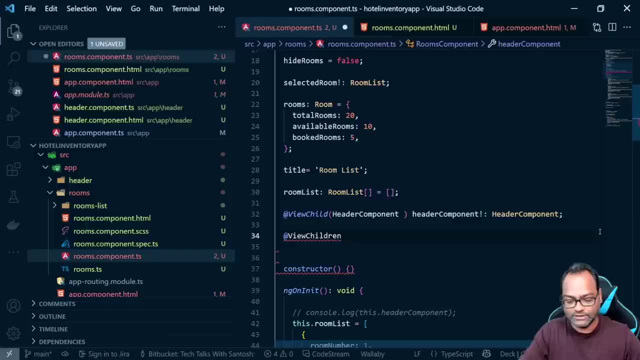 one instance, view children, in case i have more than one instance right, child children. so let's try to do: uh, use view children and the same. uh, the one difference which we have here is view children. static properties: by default false and it's false. you cannot change it. because, yeah, the same ist tactic property is by default false and it's false. you cannot change it. because, yeah, the same issue won't have an input value- default false- which, if we change this static building, you can see generation server is used and generation server screams: do object's root. so if you change this, Part 0 puis. 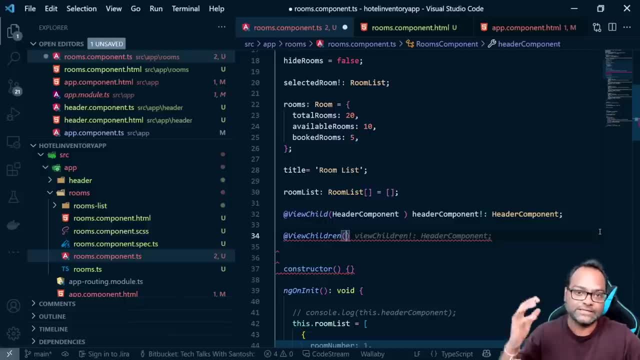 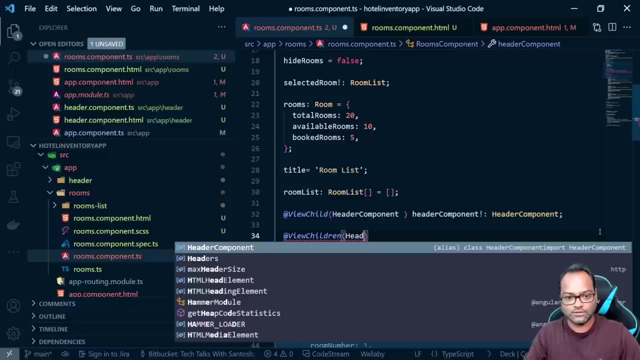 is 2019 minus 204, which means now it Siemens the other variable which we have right. so let's change this part which you can addacon. two side is false. you cannot change it because it is saying, okay, you are going to have access multiple instances and it cannot be available during ng or init. so here i will pass header component. 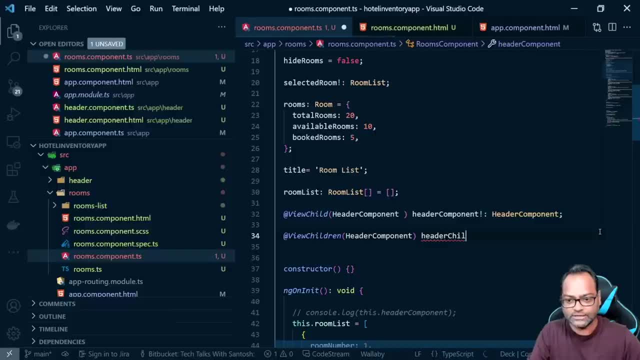 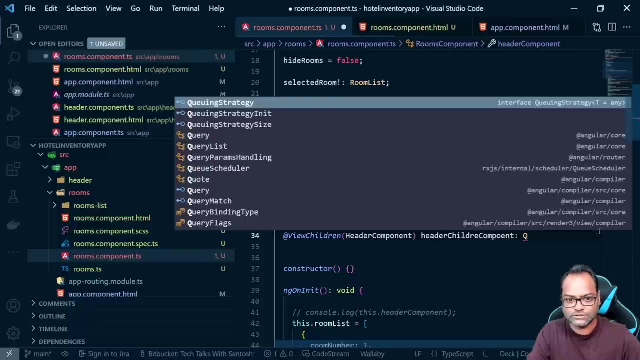 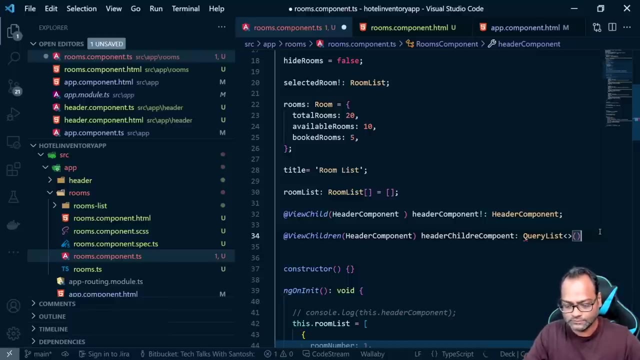 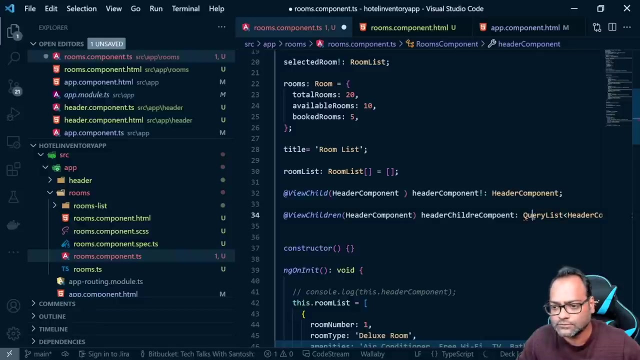 and here i will say: this is header child, children component. and we have to just do one more thing now: query list. so let me just write this code and then we'll talk about it. let me see, query list is imported from the correct path. okay, it's still not. 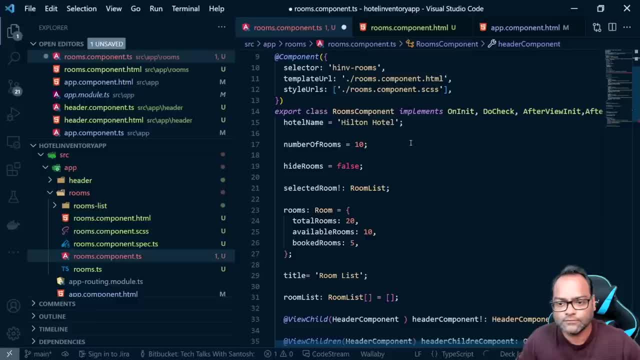 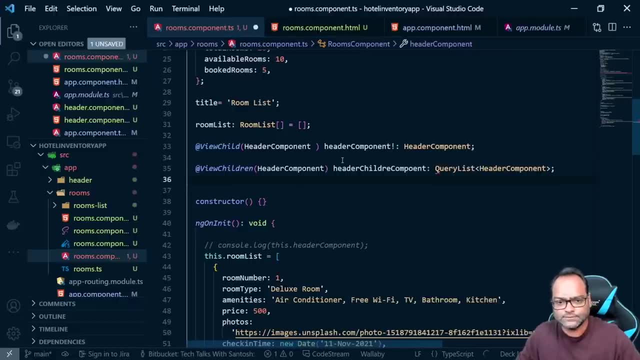 let's try to. so we have this, uh sorry. so we have this, uh, view children, and we are saying this is the property and this is either children component, children component, and we are saying this is type of query list of header component, what we are trying to do here. so let's see, let's see. 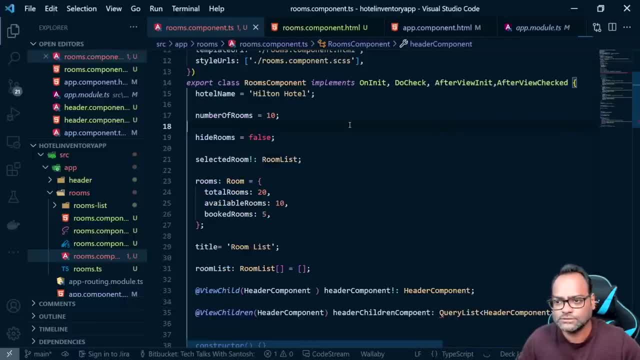 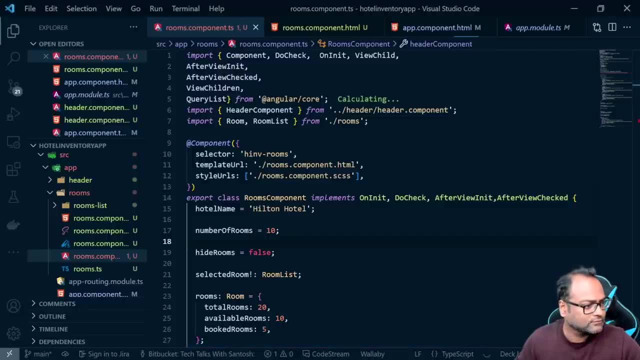 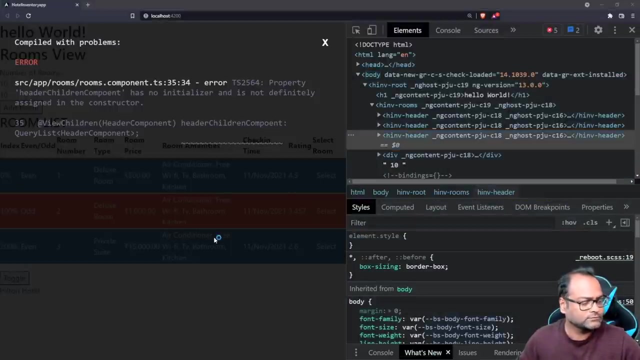 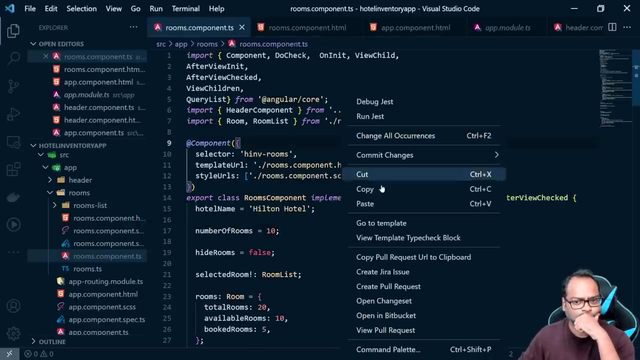 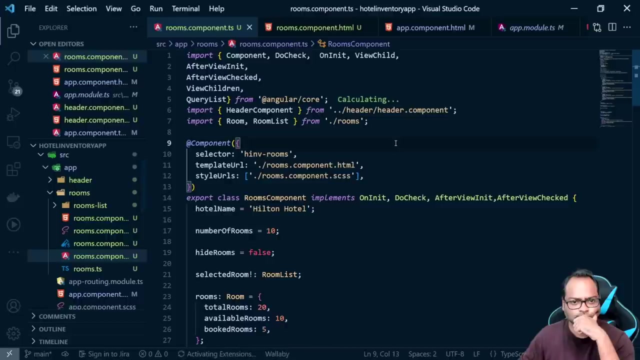 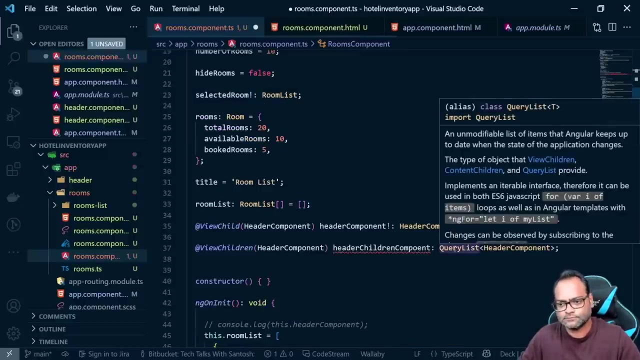 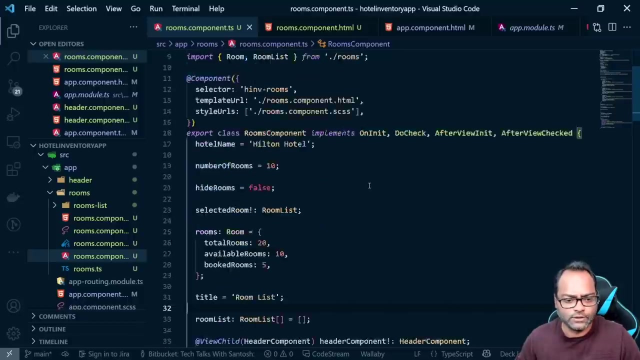 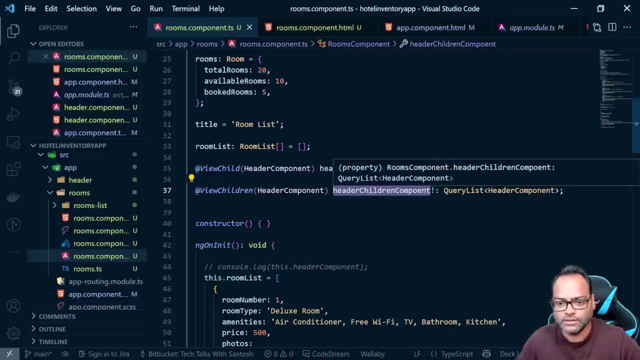 okay, looks like my laptop is consuming a lot of resources. so i will say it, the key we have is my- so you know i- or other activities. okay, so now here. so what we did is we created, we used view children to create instance of header component and then we named it as header children component. 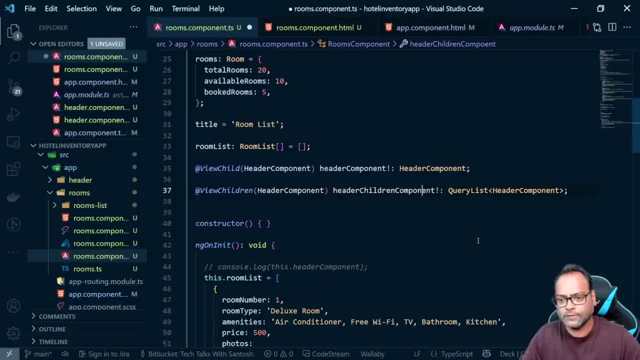 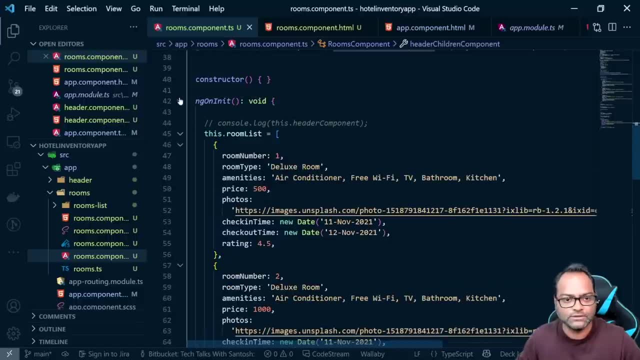 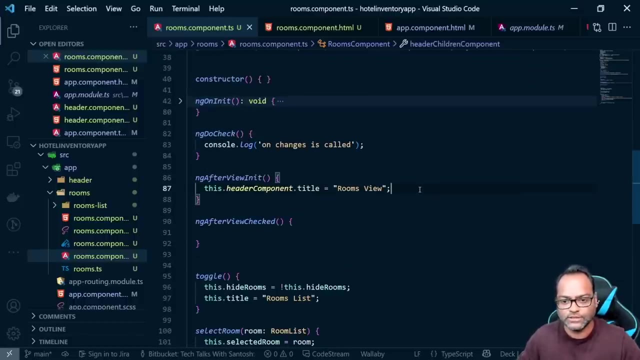 and we just type of query list of header component. let's try to just to consolelog and see what what happens here, and we know that we cannot access it inside ng on it, as we said, that is like static is false by default. we cannot do anything here, so i'll set this dot. 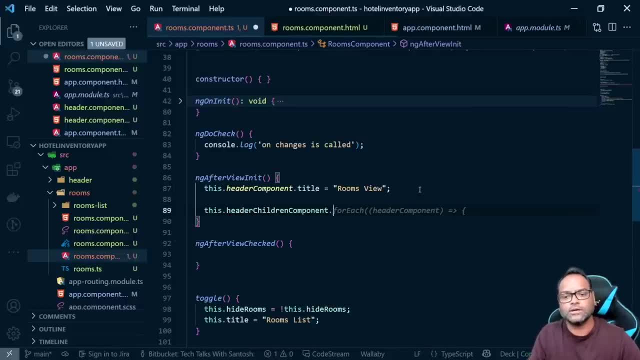 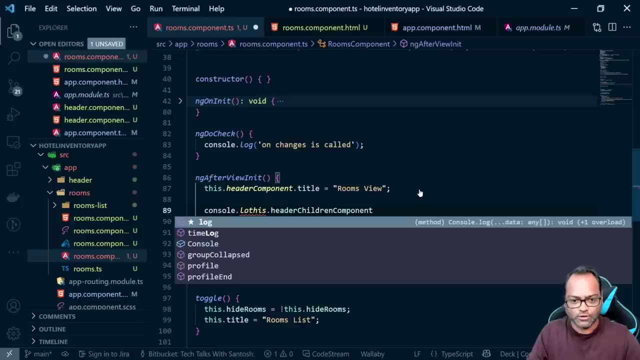 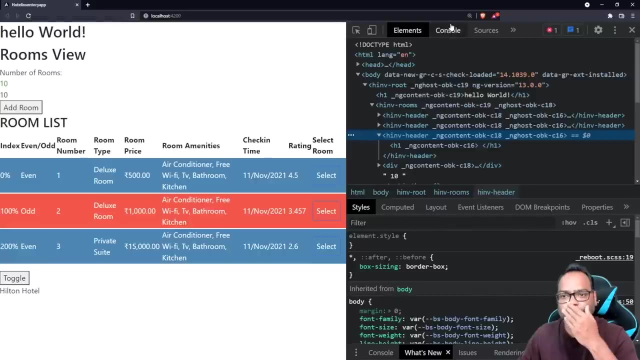 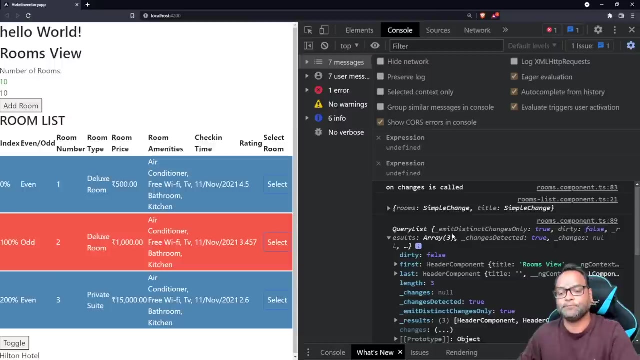 uh header: children component dot. now you can see it says forage. why it is saying forage? because, uh, let's do consolelog and then we'll see what it contains and then we'll talk about the properties it has. okay, so you can see, uh, what uh it has. it's a query list. it has a property called dirty. 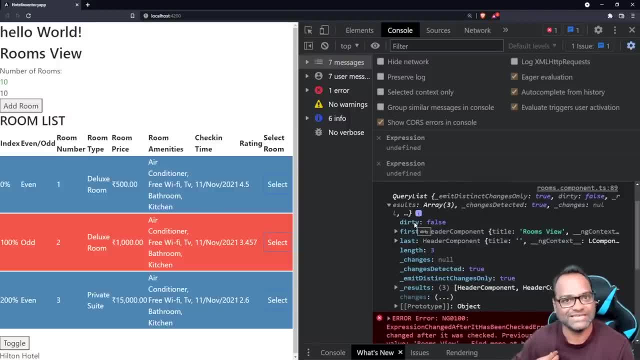 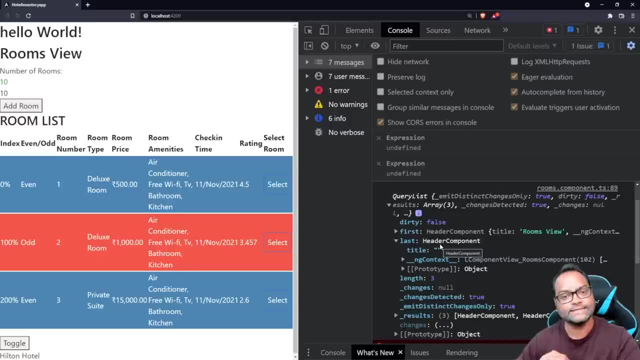 it means dirty, means there is no, uh, nothing has changed inside this particular component, then it has first and it has last. this is first instance and last instance. so in case you have like multiple components of same type and now you want to do something different with first instance and last instance, you can do that. for example, let's say: uh, you have, you, you have. 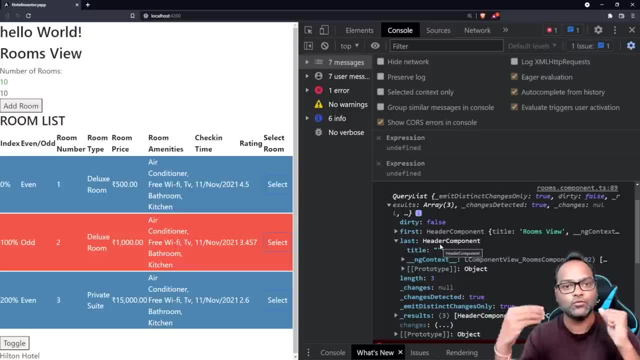 multiple rows, like, let's say, you created a component and you want to render them as rows. you want to take first row and show them as header, take last row, show them as footer and whatever is in between. you can actually create a, create it as your content. that's possible. 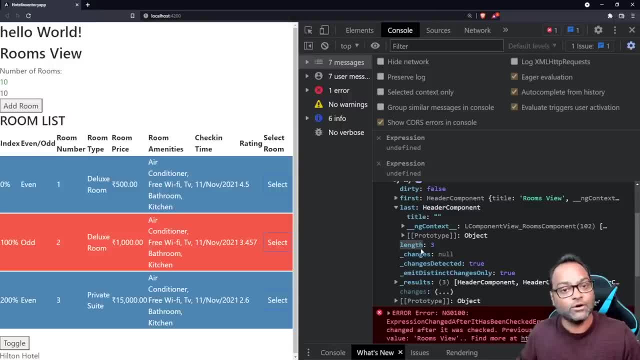 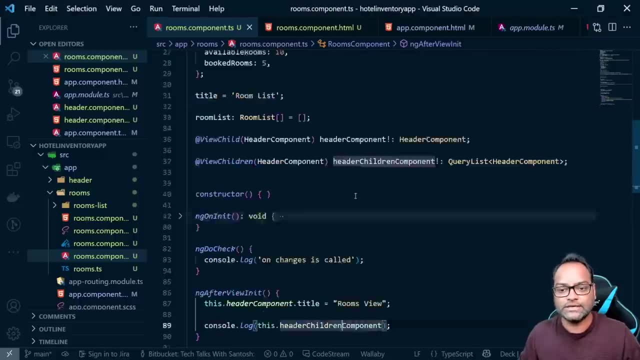 using first and last. you have also length property, which tells you how many results are there, and then you have underscore results property which gives you all the result. so it means it is an array. so query list is something which has access to all uh properties which is available here. 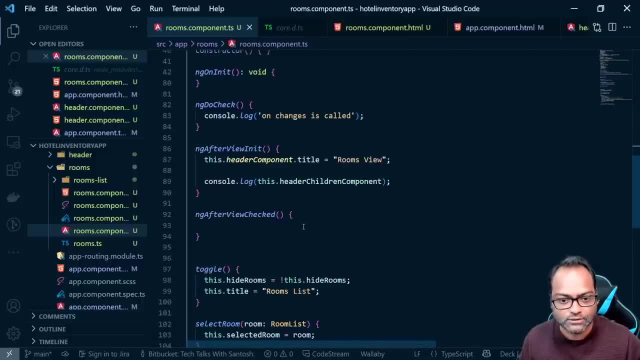 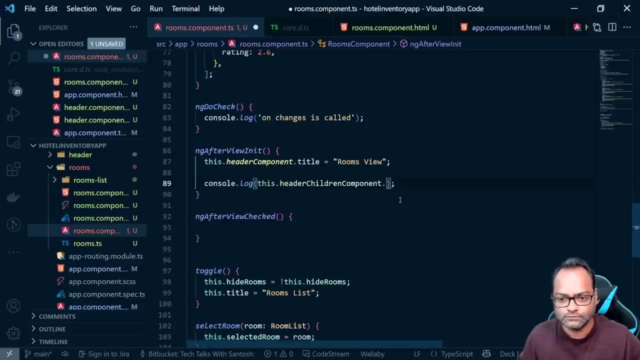 you can, uh, let's go ahead and see here, right? so i can just go ahead and say i had a component dot last, and so i can access last component, and then i can access the title property of last. so i'll say: this is uh last title, just random string, right? 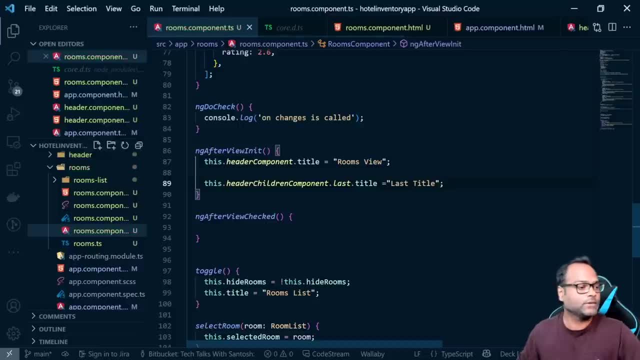 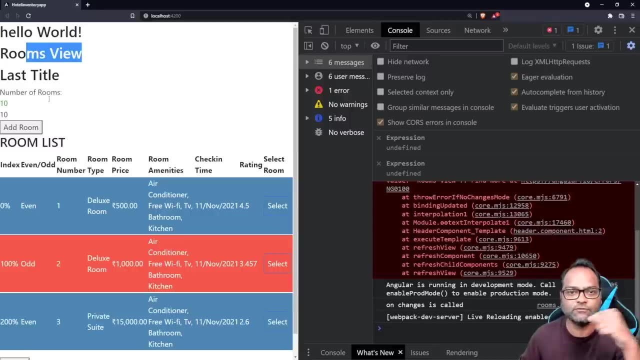 and let's see the output. so it's a. it says: okay, this is your rooms view, which is first instance and last instance, and then i can access the title property of last instance, which we have already changed using view child, and this is your last title which we changed. 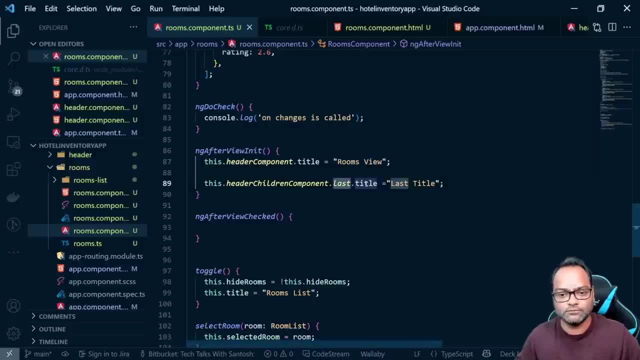 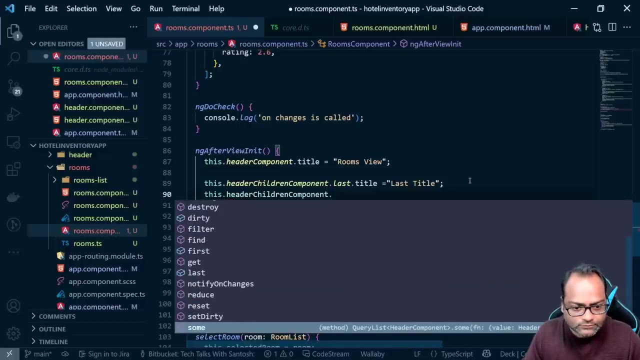 using the last property. in case you want to do, uh, something with each and every row, you can actually do it by using for each loop and what else, and we will see not different changes later. but yeah, i mean, this is like an array, so you will get all the methods, most of the methods, not all methods which is available on. 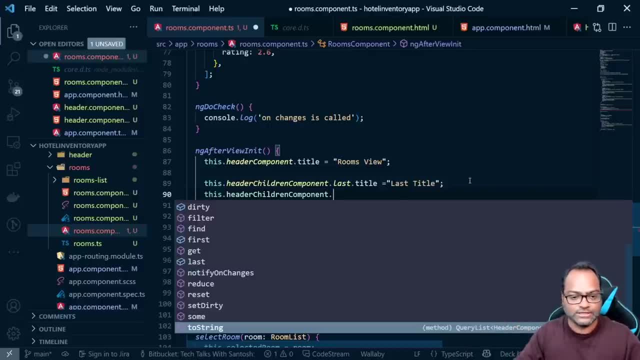 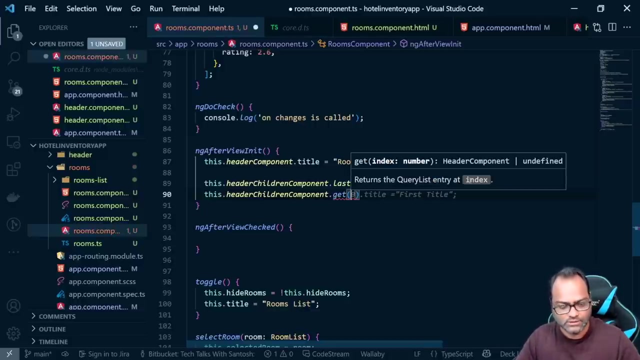 your on on your array so you can see it has some. uh, there is something called resect, but and it's not what we need, so we have fun. find filter and you can also call destroy to destroy any component. those thoughts, okay. and you can also get any um component using index, in case you want to, here you have get method as well. 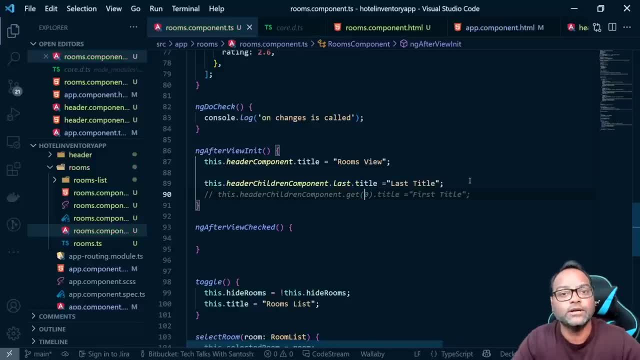 so this is, uh, what you can do using in the children component. this is really useful in case you want to create your own, um, let's say, reusable component, or your component where you want to create your drop downs right. so, where you can, your users can pass the list of records and you can display them as you want- not the user want, right. 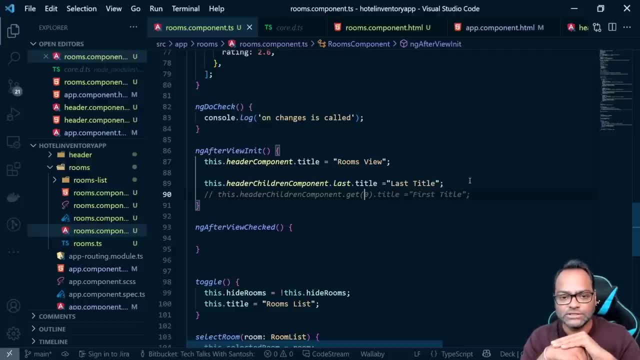 So these are some examples. Angular material uses ViewChildren at multiple places. You can check out the code base to understand it more. So this is it from ViewChild and ViewChildren. We also discussed about how you can use ViewChild, how you can use ViewChildren and the lifecycle. 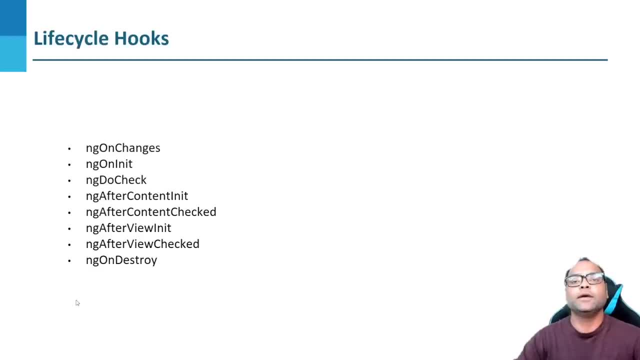 looks as well. In previous video we saw how we can use ViewChild and we also discussed about some scenarios where ViewChild is useful and ngAfterViewUnit- lifecycle- look hook as well. ngAfterViewUnit hook as well. Now in this video we are going to talk about ngAfterContentInit. 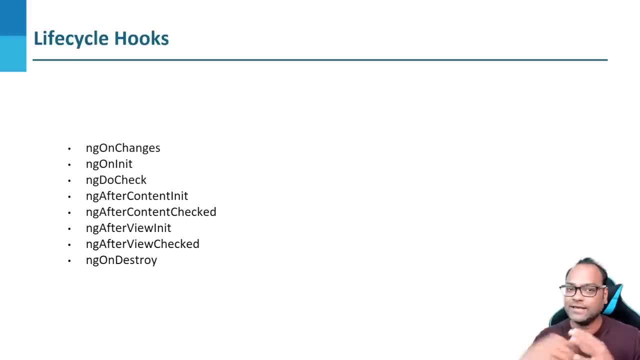 But, as I said, we will be going through the lifecycle as well as some of the concepts. So here we are talking about after content. So it has to be, it has to do something with content. but what content we are talking about? 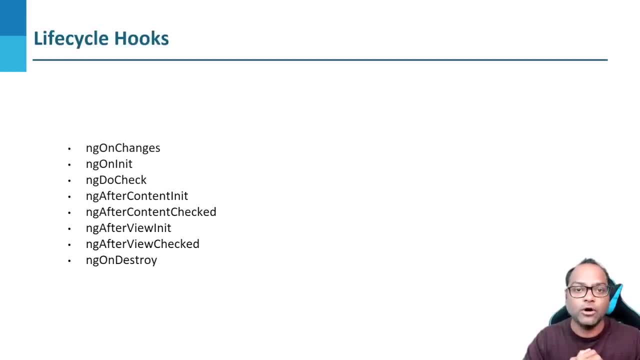 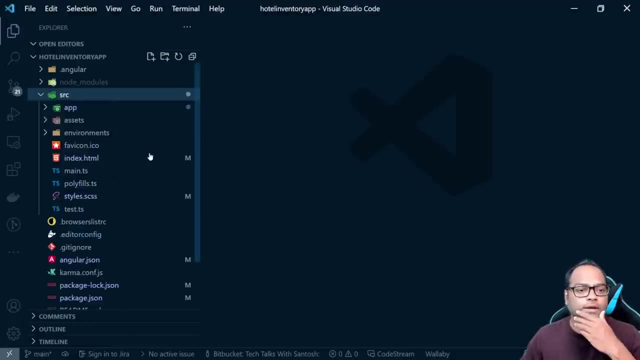 Here we are going to talk about a really important topic called content projection. So let's go ahead and talk about content projection and then we'll come to ngAfterContentInit and what it is and then how we can use it. So let's go back to the code base and for this what we will do is we will create a 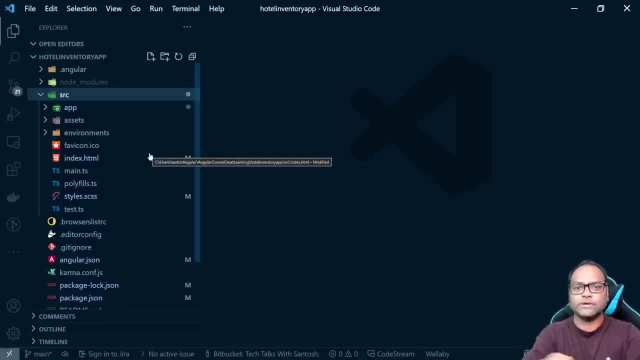 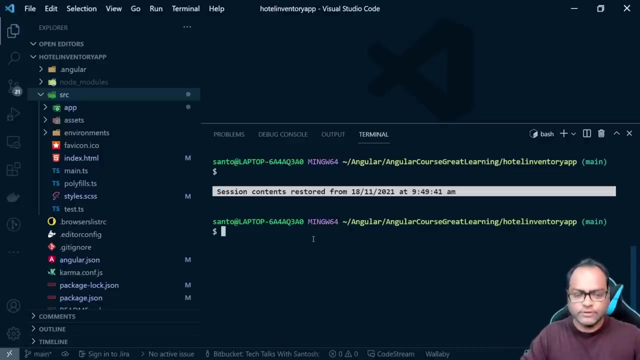 new component. So, because we need to understand what content projection is, so I'm going to create few components and then let's see, let's, we'll talk about the content projection. So first component which I will create is, let's call it as container: 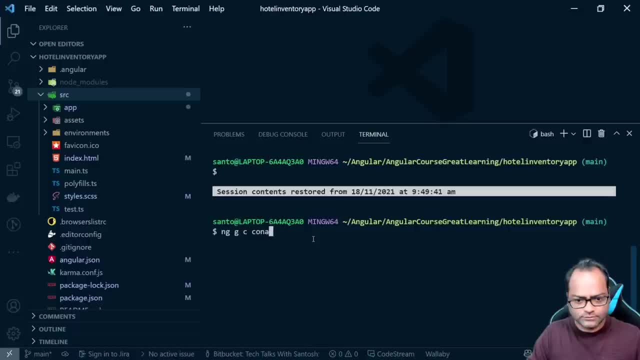 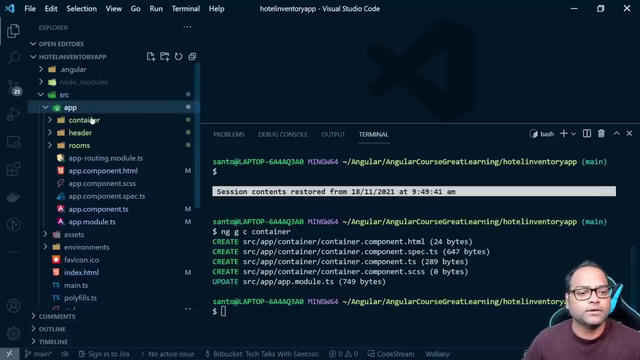 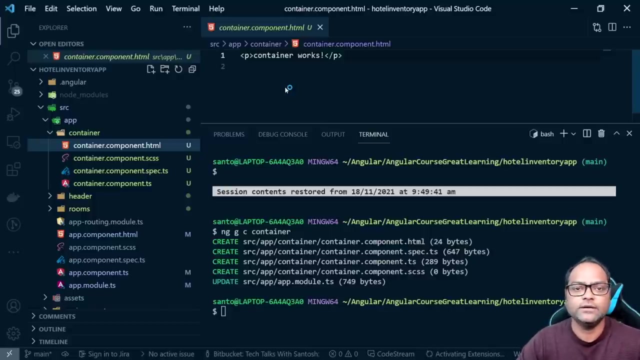 So this is a container. So this is a container, Okay, Okay, So this is a container component, and why content projection is useful. let's talk about once we create this component. So let's say, you have your application right. 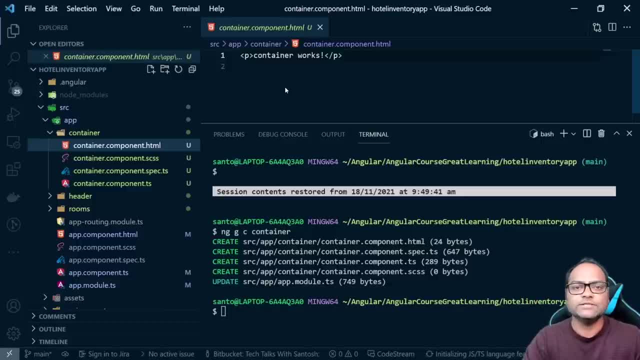 But what you need is you, once you finalize your design system, you said, okay, my sidebar can be on left side, My footer can be on the lower side, My header will be on top. Okay, So this is the top of the top of the page. but use, I don't want to actually give this. 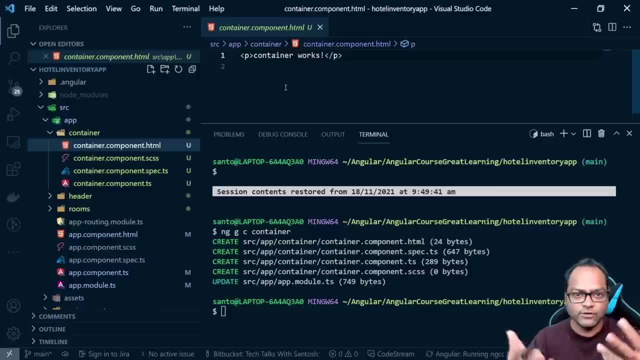 functionality where user can decide. I mean not the end user, but my developers. As a lead engineer, I want to actually take care of where the components will be rendered and in what sequence. This is where actually these are few scenarios where this is actually one scenario where 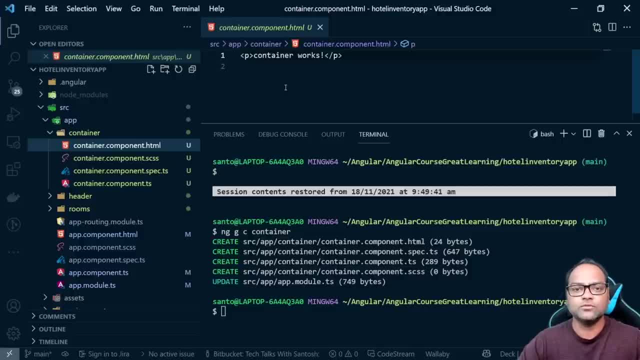 content projection is useful. What else? You have created one component, As you said, components are, of course, your reusable estimate tax. So what we need is: we want to give that reusable estimate tag, but what content should be placed inside that particular container or a particular component should be defined by user. 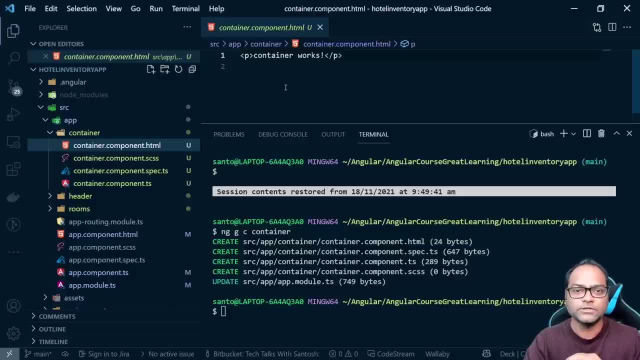 Again, if I talk about user here, I'm talking about the developers, So your developers should be able to define that. Okay, I want to put some, let's say, as one tag, or I want to put a break here, or I want to. 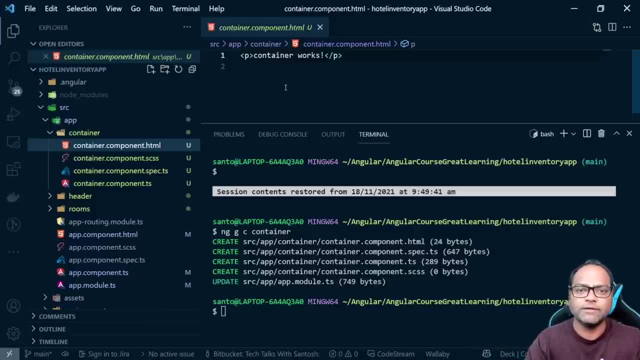 put a horizontal line here. That's something which is up to the developer. So these are two scenarios where content projection can be really useful. Let's go ahead and do that. So, first, how we can achieve that. So, to achieve the content projection, what you have to do is you have to place an HTML. 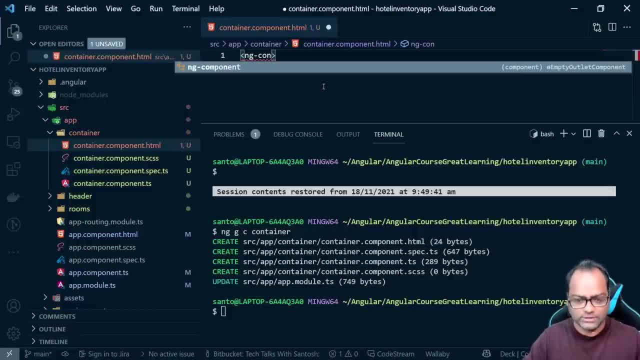 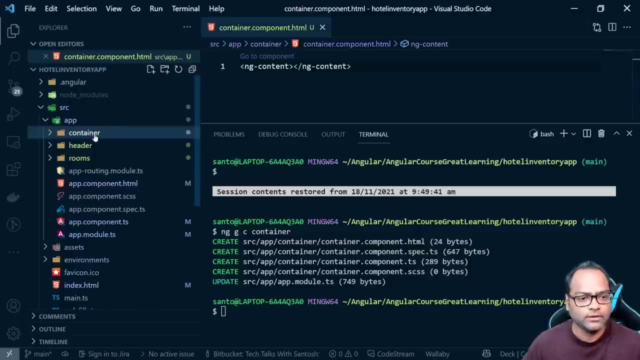 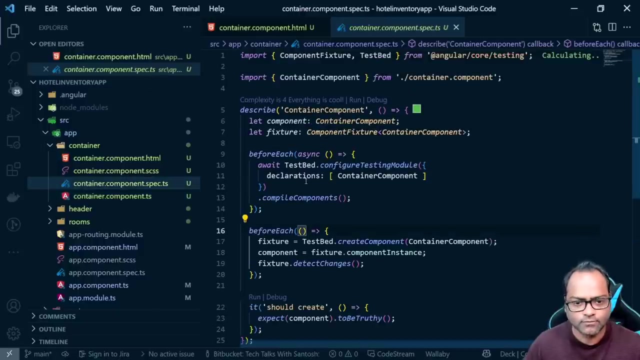 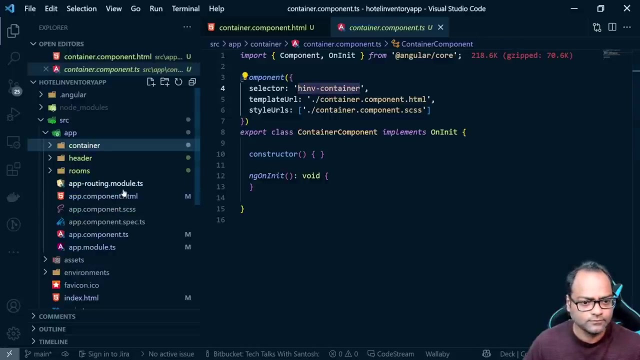 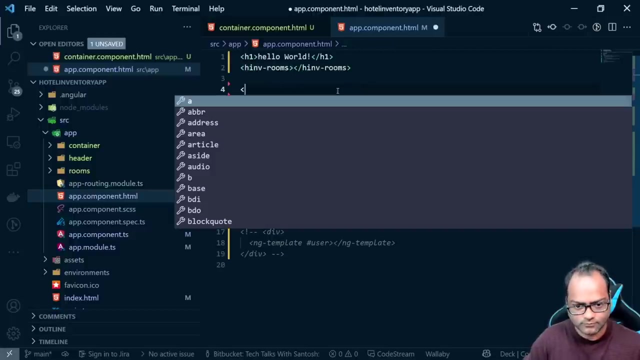 tag called ng-content. So let's do that and say ng-content, And this is what we have. So we have ng-content- open, closed, that's it, nothing else. Let's take this component, let's close this. So you might be wondering: why are we doing this? 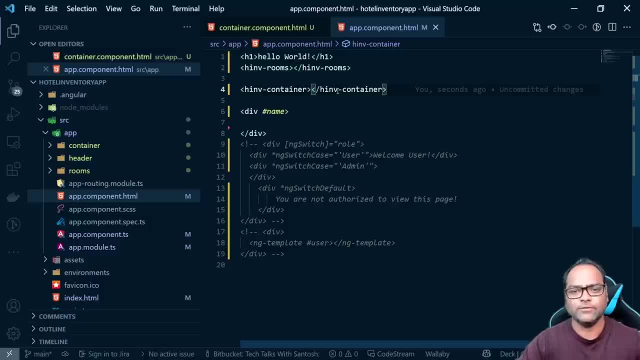 Why are we doing this? I think what is different here? I mean, we have been doing the same thing earlier as well. right, For example, rooms component. we have placed a room component open, closed. that's it How this ng-content is going to help us. 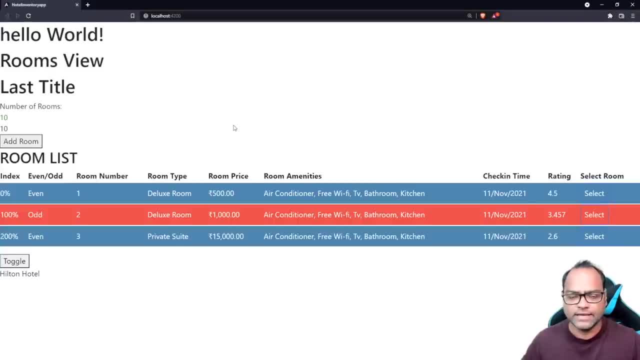 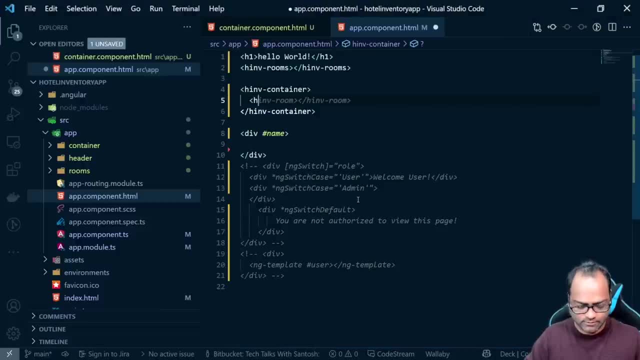 So let's see the view It is as it is. Now let's try to put some HTML contents here. So what I'm going to do is I'll place an h1 tag. I'll say: this is from ng-content. Okay. 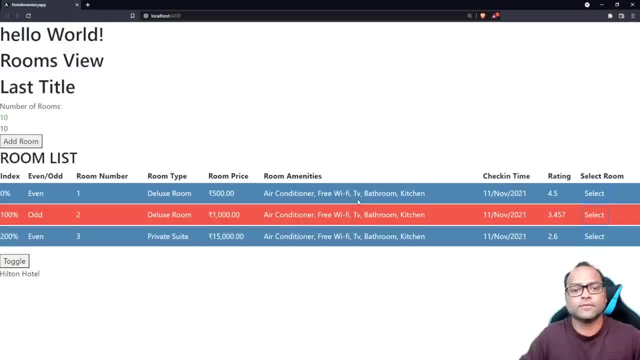 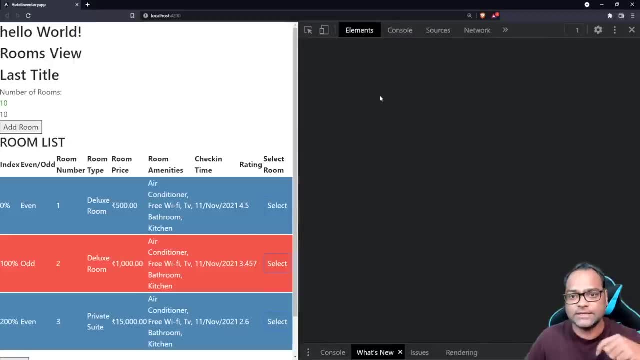 And you can see you have this is from ng-content available here, the content which we placed inside an HTML tag And if you see this, I mean, of course, this is how it looks like: h-i-n-v-container, and. 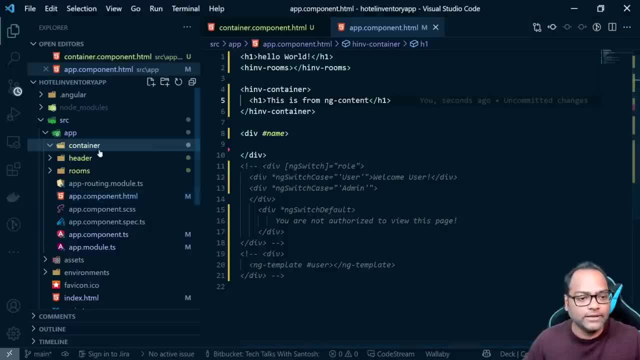 then this h1,, which is replaced by this ng-content which we have placed here. So it will not work with other tags, For example, if I do try to do it here- for example h-i-n-v-rooms, we don't have any ng-container. 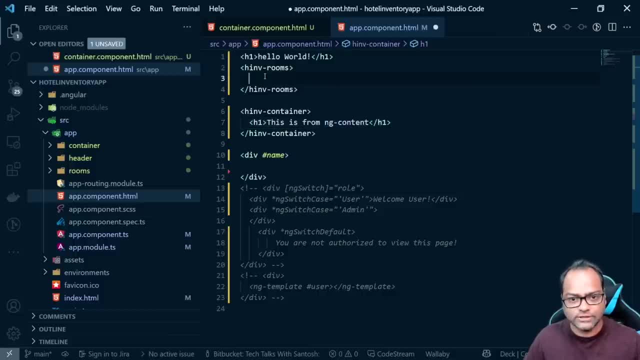 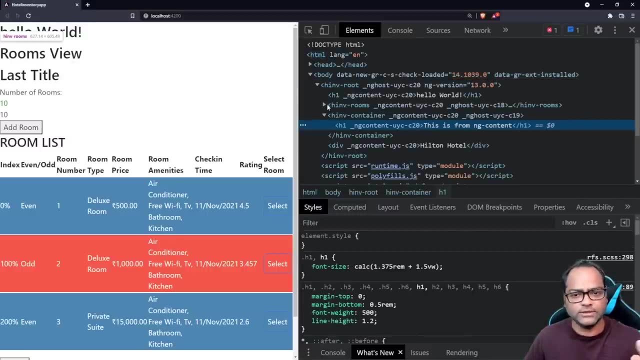 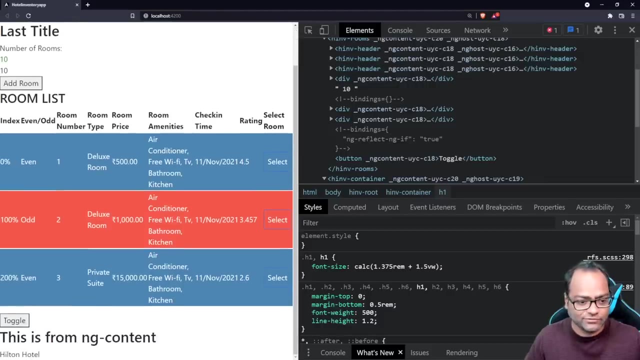 here, So it doesn't know what to do with this. So let's go ahead and try this out and see. And you don't have anything here, right? So in rooms you are not getting that particular h1 content which we have placed. 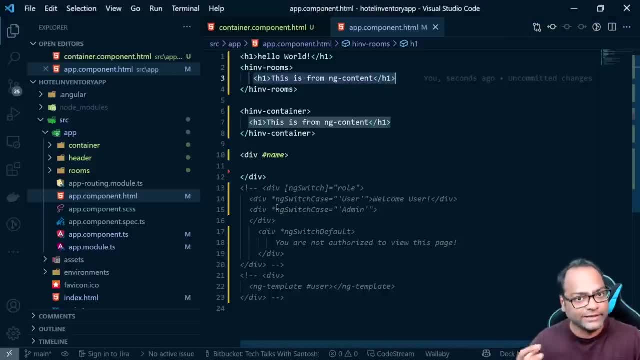 But here we are able to get it because we have placed ng-content and ng-content knows that. okay this. so there will be some content which will be passed by the user. I mean, as a developer, I mean, you can be. 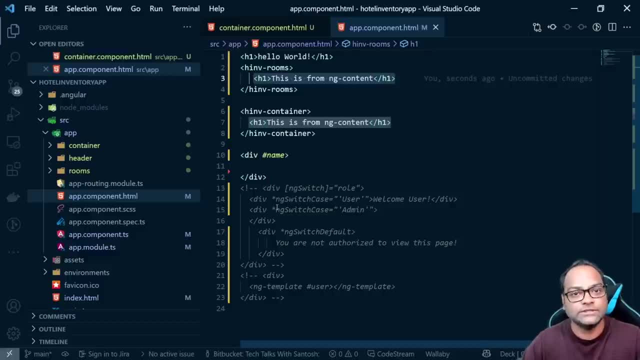 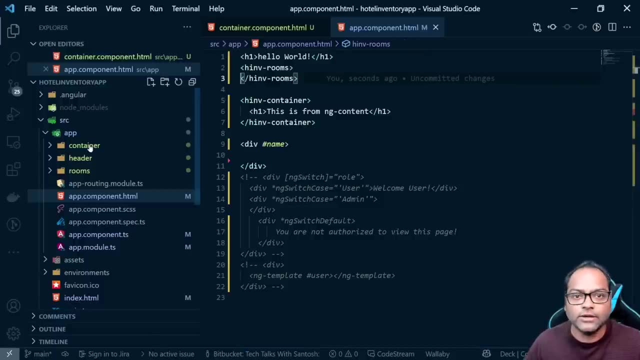 The same developer, right, You, who is writing container and who is using that container. So this is what you can achieve using ng-content, but of course, this is not it, So let's go ahead and talk a little bit more in detail. 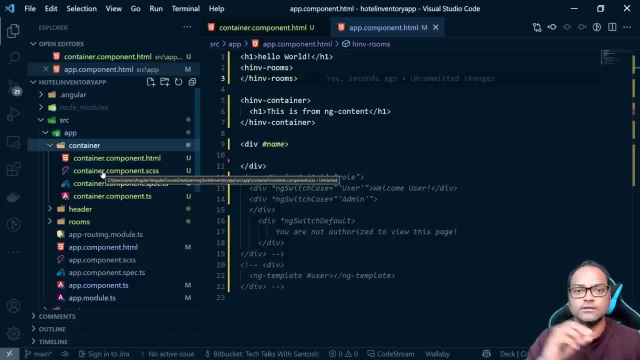 You can also do one more thing. As I said, you can provide the order in which you can. you want to actually load your components. So let's say, I can give or I can create a container component which has like your dashboard. 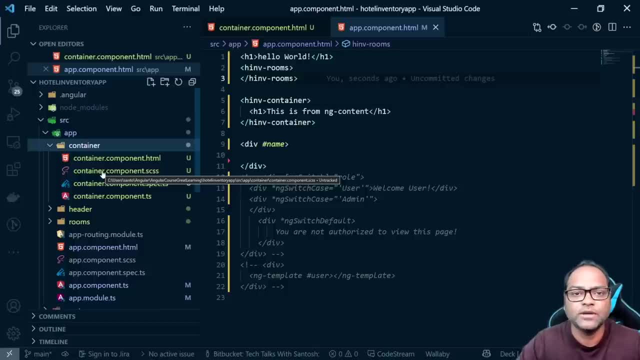 header, footer, sidebar, placed accordingly right. But you don't want to actually do it by yourself. I mean, containers should not have anything. So containers should define: okay, where goes what? that's it There isn't me. Let's say what you can do is that container component is, let's say, is your reusable component? 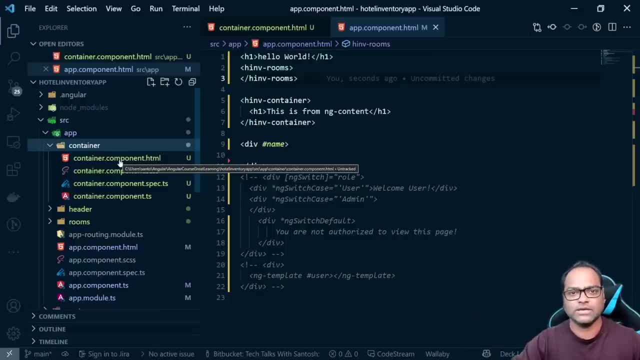 And now you are going to use that reusable component and across multiple applications. So what you have to do is you have to just create the component and you have to just place them. That's it. That's all you have to do as a user, I mean as a developer. 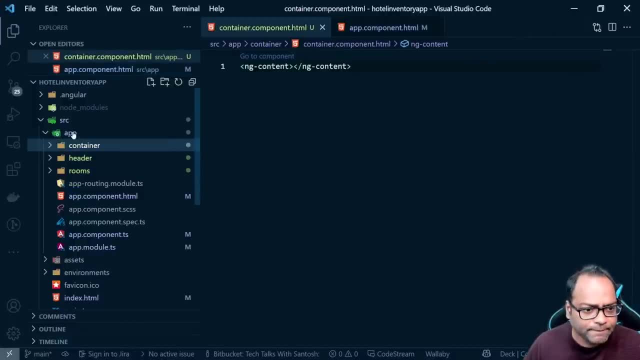 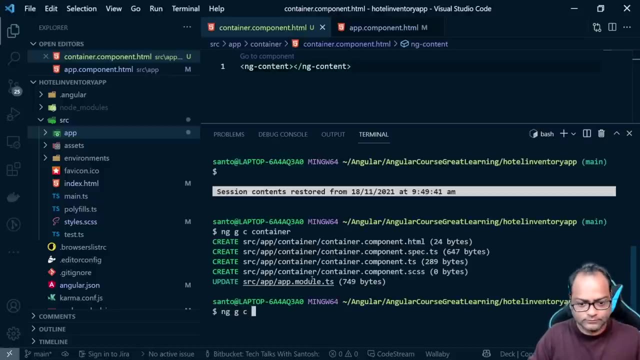 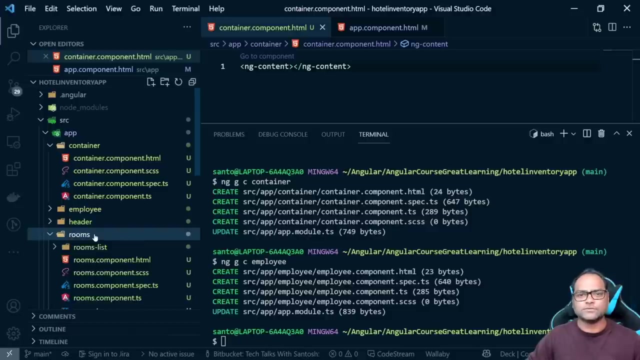 So let's create a few components here, Let's see what we can create. we can create an employee component, So of course hotel will have employees And we already have rooms. So we'll these are two. So let's say now what I want to do is I want to load, let's say, employees data first. 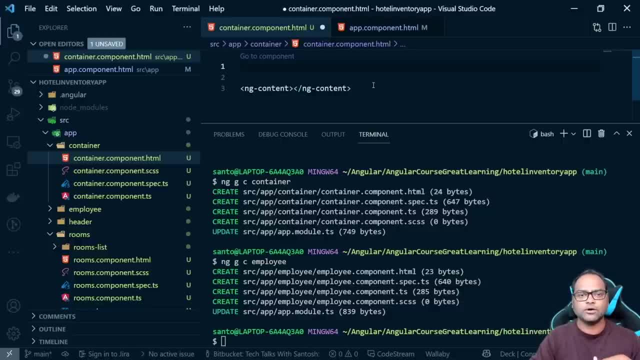 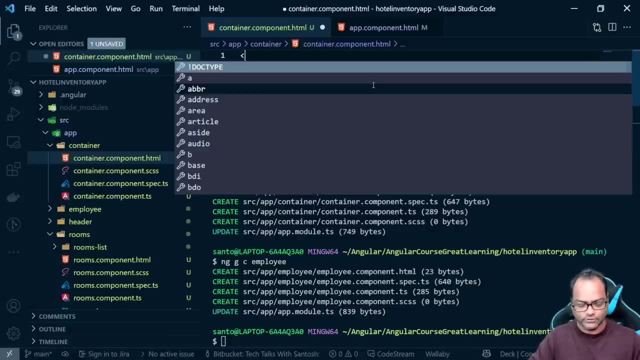 Then I want to give an ng content where people- sorry, where developers- can add whatever content they want to, And at the end I want to load rooms. So let's see how we can do achieve using ng content. So in ng content you can. 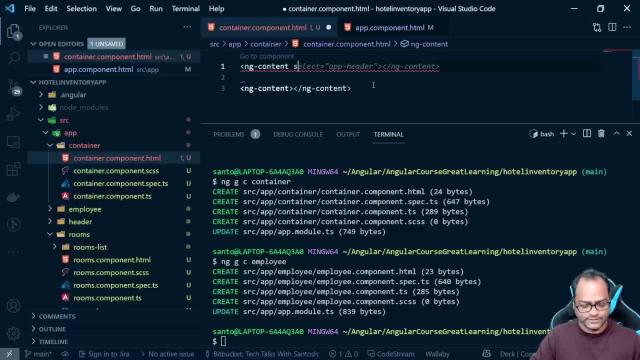 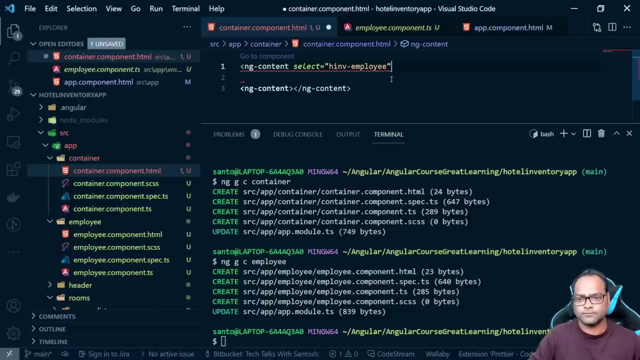 Okay, Okay. So in ng content you can pass a property called select. In select you have to pass the HTML tag. remember this. So first, what I want to do is I want to actually load employee. So this is where I'm going to place employee. then there is an ng content. 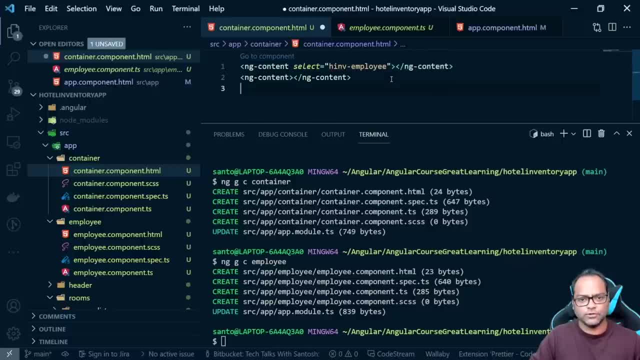 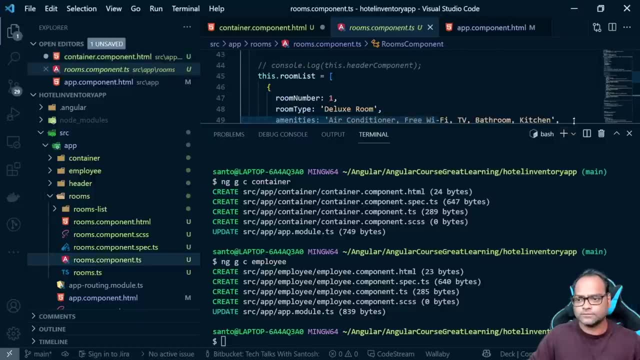 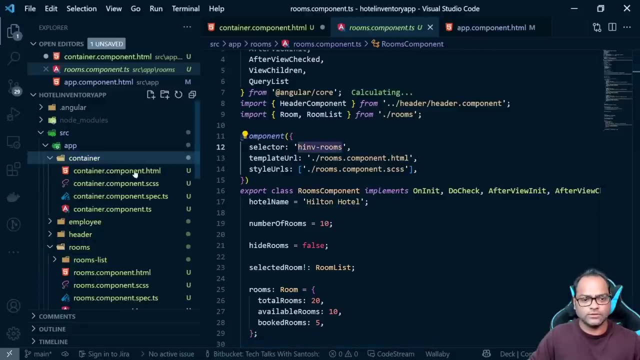 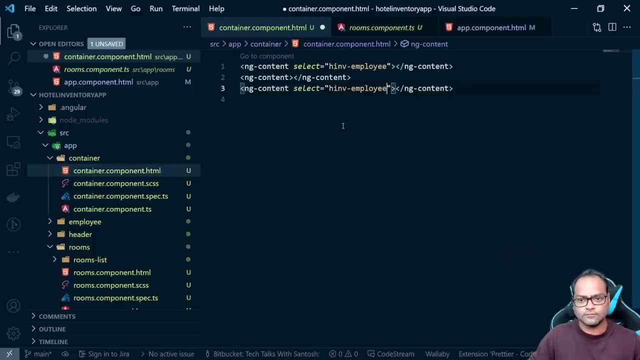 And at the end, what we want is: we want to load rooms. So let's go back to rooms, Let's close this again. take rooms, put a container HTML and let's replace this here. Now we are done with our container. 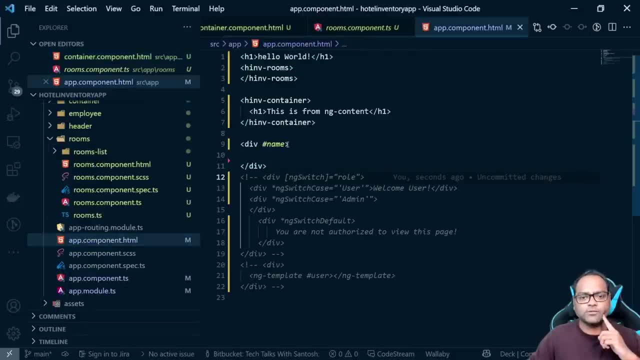 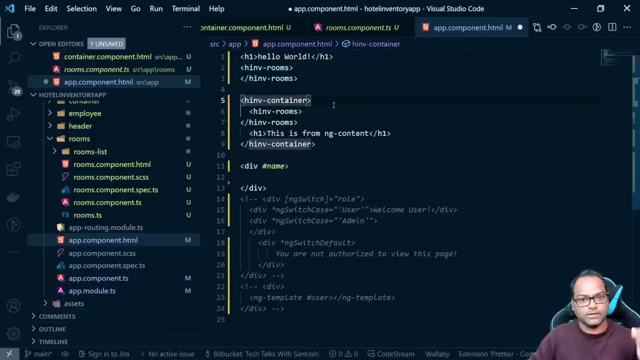 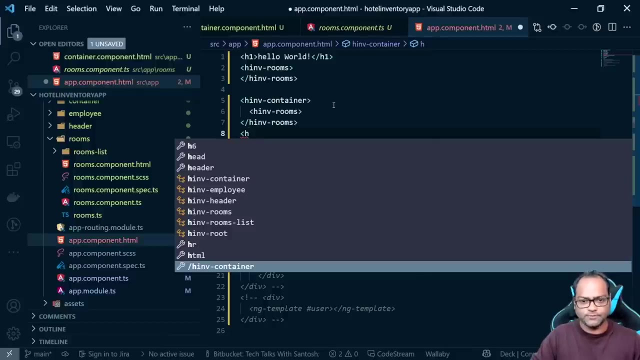 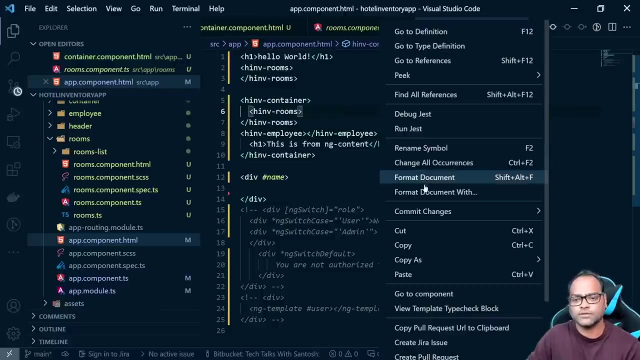 Now let's go back to this main componenthtml. Okay, We have this container available here, So what I can do is I can place. So remember I'm placing rooms first and let's put in employee second, And let's save this in this format. 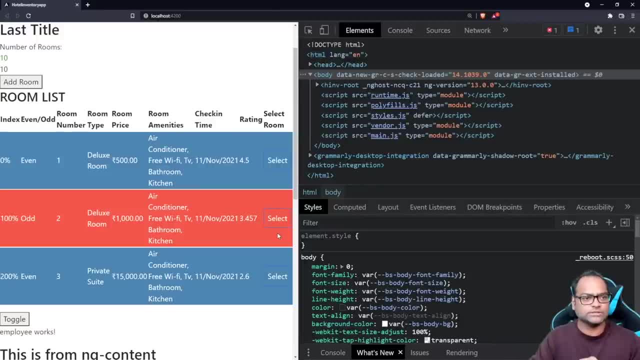 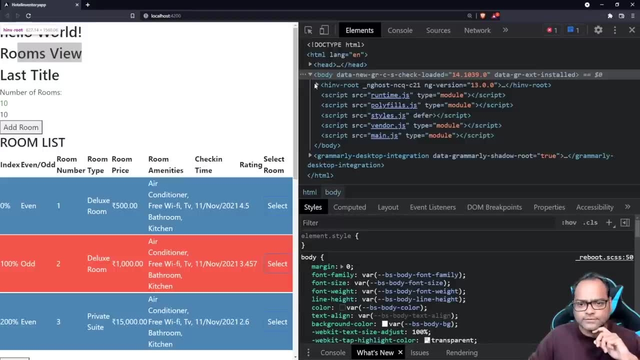 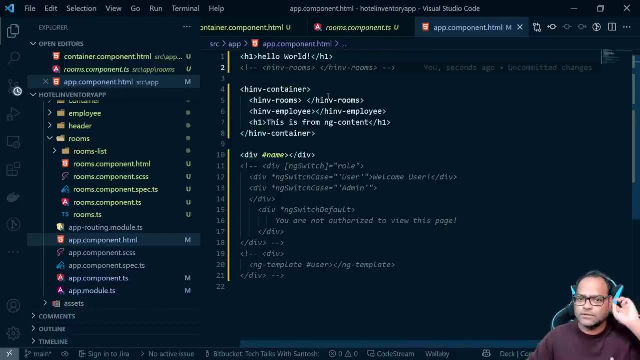 And let's go back to our page. So this is, this is how it looks like, So you can see. You have hello world, then you have rooms view and let's see here- I need to comment this out, Otherwise rooms data will be like displayed twice. and let's so we it's compiled now you. 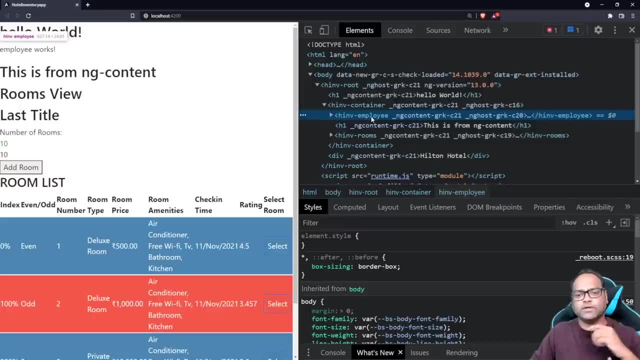 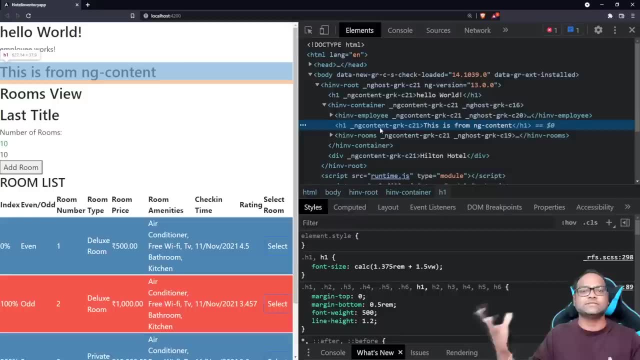 can see. So let's open the container. You have employee first, then we have: this is from ng content because we placed an empty container. We are saying that okay, whatever doesn't match comes here, And then we have rooms. 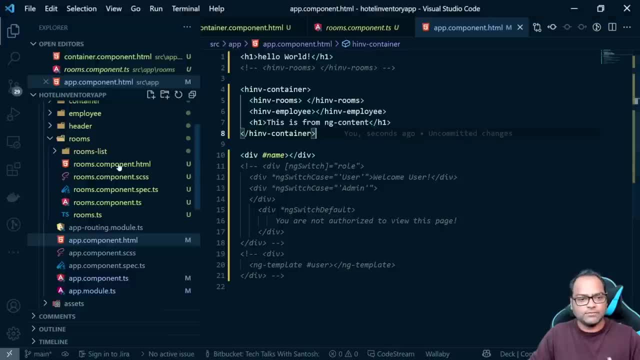 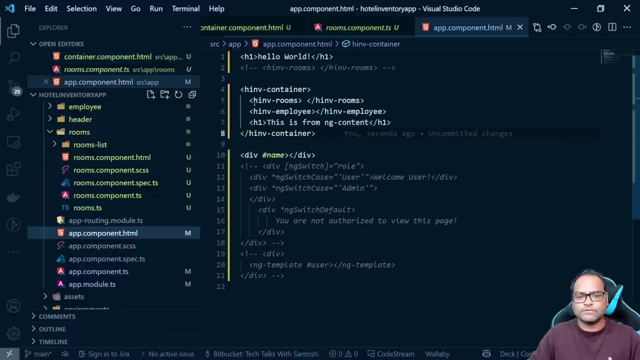 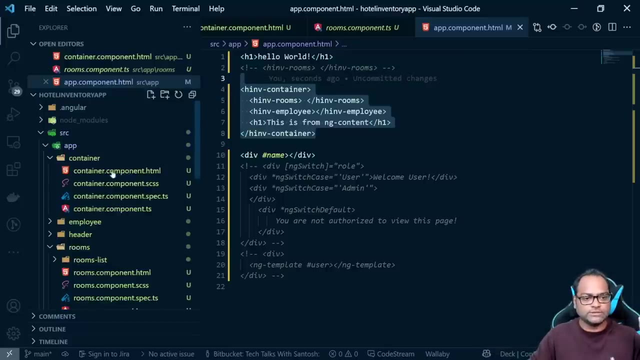 Okay, And we don't have the same sequence Here. I mean, we we don't have same sequence here. We are loading the rooms first, employees second, and then at the end, and doesn't matter, I mean because you have defined this. this is the sequence in which I want to actually 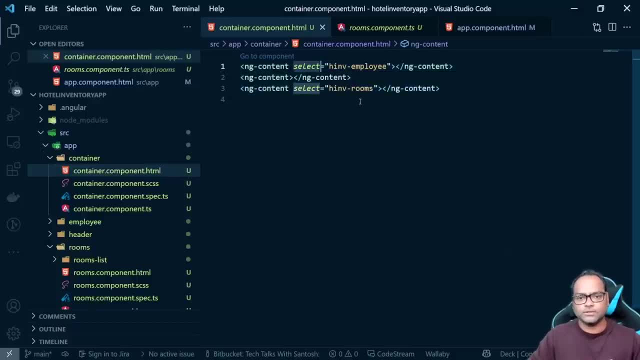 load some content And you have also defined these. these are the matching tags. So select. we are saying okay, select this particular HTML tag or select this: Okay, That's fine. Okay, particular component, right, which will be placed here. so this is how you can actually use containers. 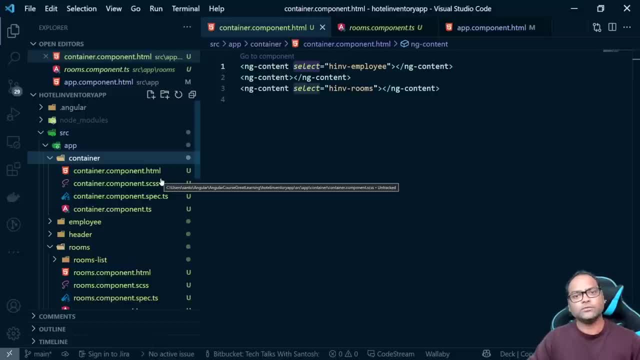 now what else, what else we can do? we are talking about ng con ng after content in it, now what is the content for a component? so for this particular component, if you talk about container component, the content is something which will be loaded or which will be provided by the parent component. 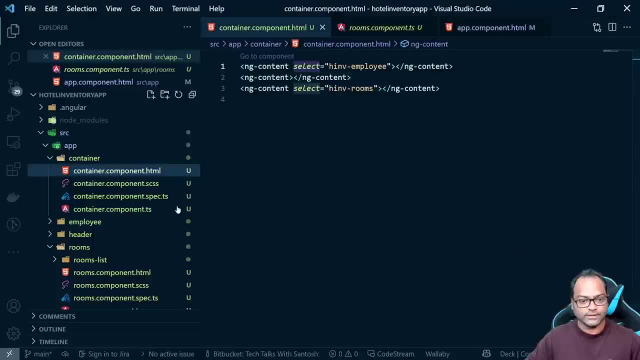 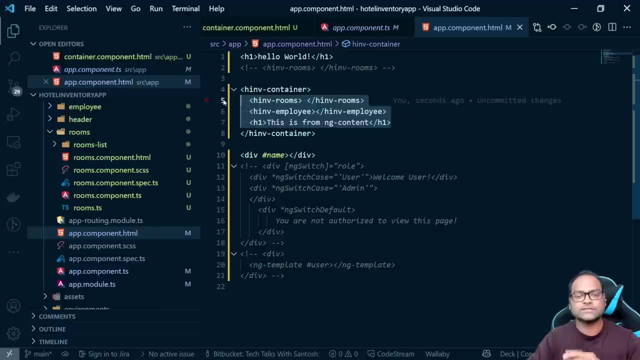 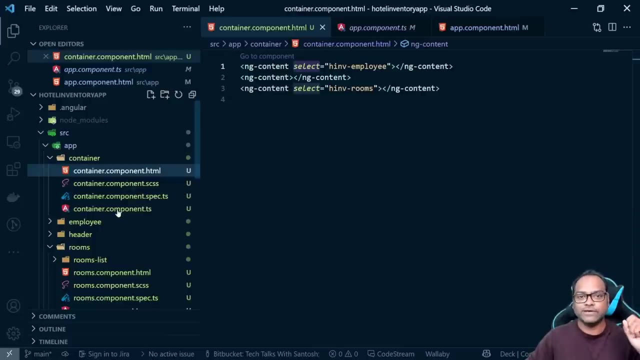 so that content also, whatever is loaded inside this container, is the content now your components. so my container component can only access these components in case they want to inside a life cycle called ng, after content in it, because at that moment the component knows that my component, my, sorry, my. 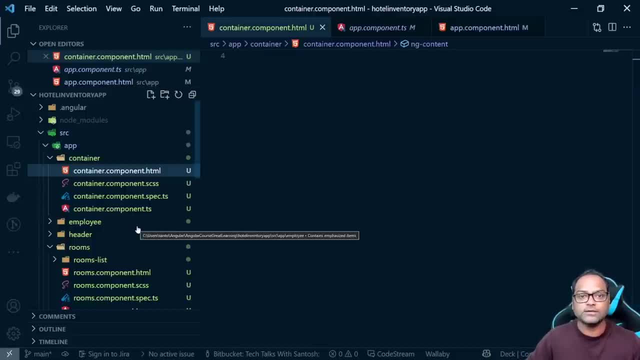 contents are initialized. so who is giving the component content? it right now it is. it is parent component, like app component, which is giving the content. when come container component will come to know that, okay, all the components are. all the contents are initialized within my component, at the container or, sorry, ng after containing. so let's put an implement and let's see what we can. 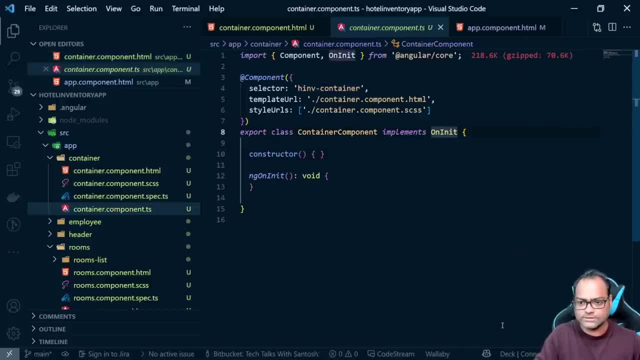 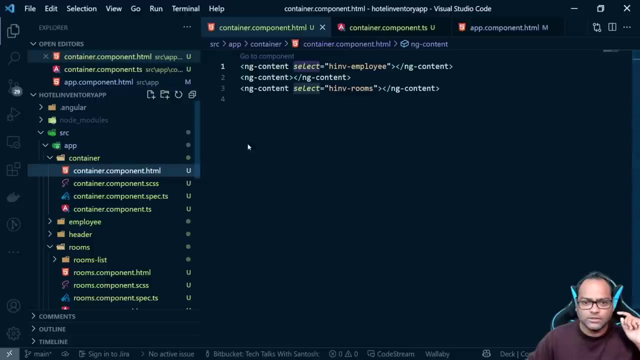 do using this. so let's say implements after content in it. and let's implement: so here you can see ng after content in it. but how to select the components? so here i want to actually select. let's say, uh, employee component, for example. let's add some properties here. 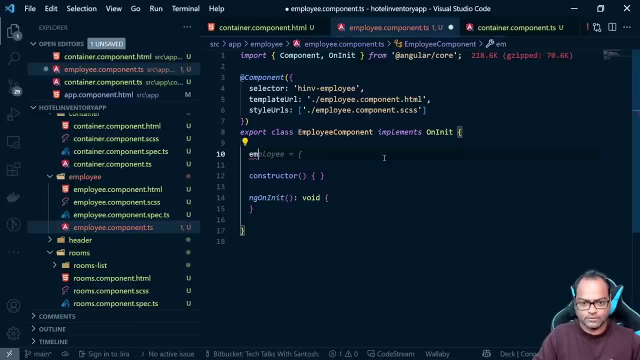 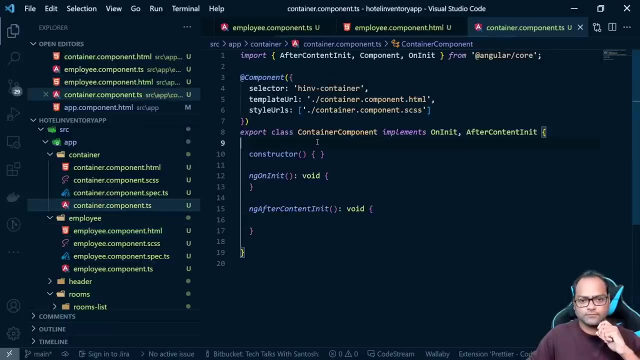 so let's say: this is mp employee name, which is string, and by default john, and let's display this employee name here. so we want to actually uh, let's say uh, access the employee component here and then probably want to change some data or want to call some action or want to actually do something with employee. 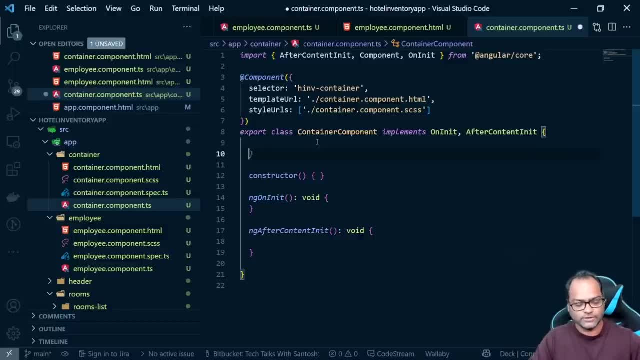 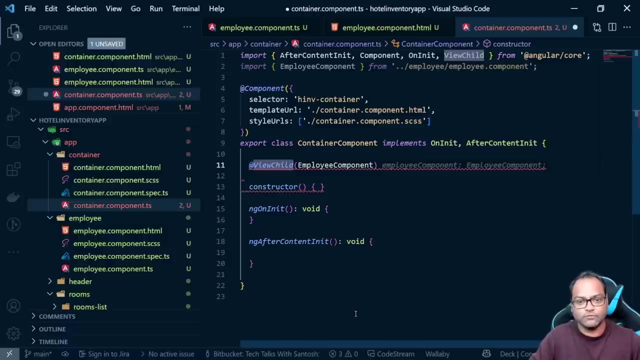 component, everything is possible. so how to access that particular component? first you have to use something known as view child. okay, so you can say view child, and then you can pass the component so you can say, okay, this is employee component. and then you can give a name: sorry, not view child. 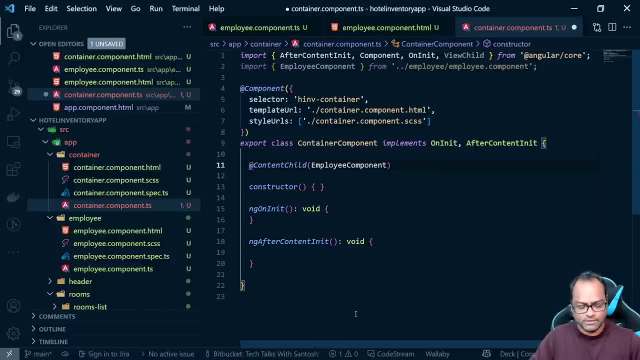 content child, so we can give a property name, so i can say: this is content component, or we can just call it as employee, which is type of employee component, and let's import your child as a content idea and now we have this particular property. of course, this is. 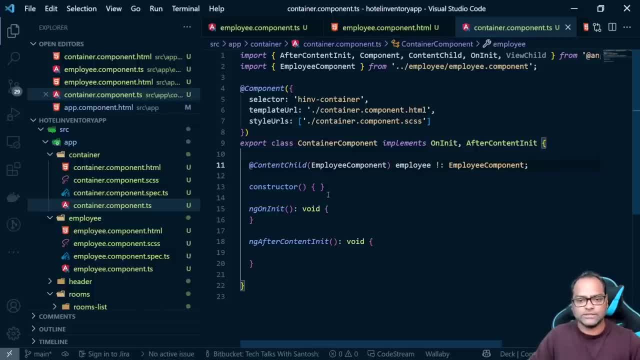 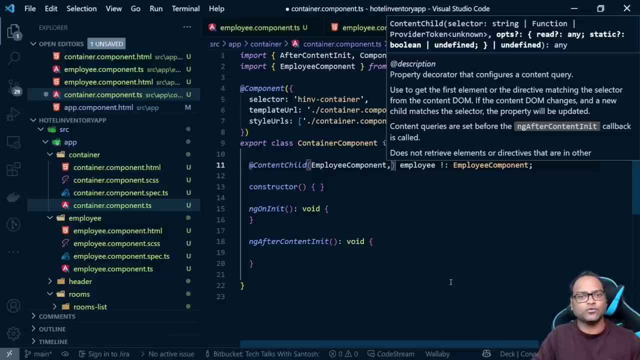 uh, strict mode, so we have to put this question mark as an exclamation mark. and now let's try to access. and uh, before we move ahead, you might have this question. so, uh, do we have static true or false availability? or false availability? so we have static true or false availability? 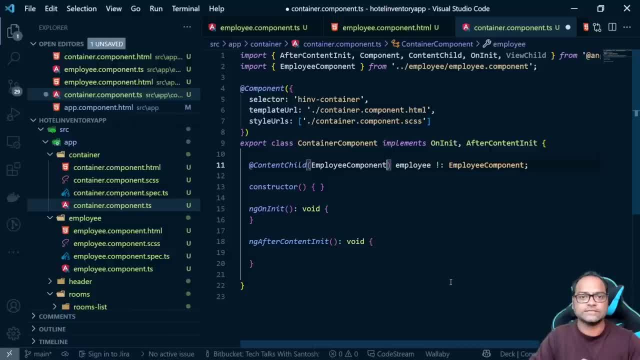 here the answer is no. uh, in content child you can actually only access those uh, everything which you have defining here inside the ng after content. so there is no option of all calling static true. there is a mean, of course, because this component doesn't know what is supposed to be. 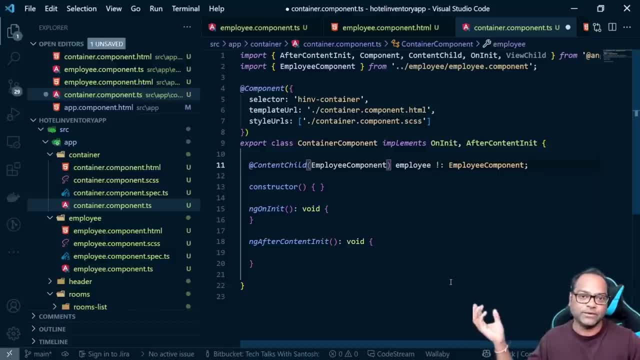 available here. it will be always passed by my parent, component and parent. it will take some time right. so running through all the lifecycle initializing its own content, then, uh, going to child component, initializing that and then coming to the content in its lifecycle- look, so it won't be available. 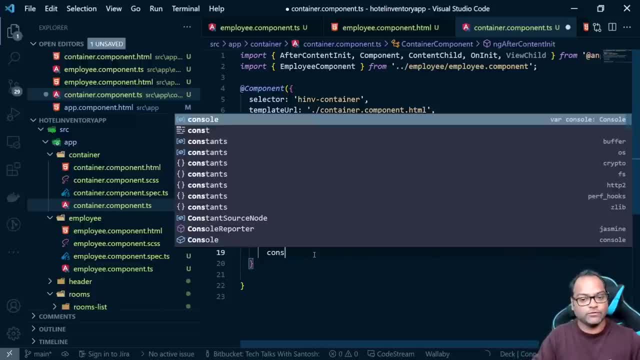 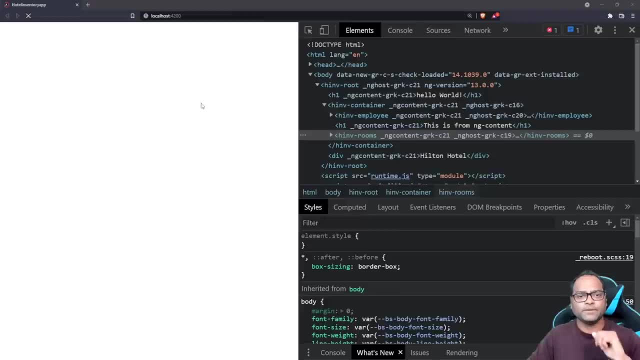 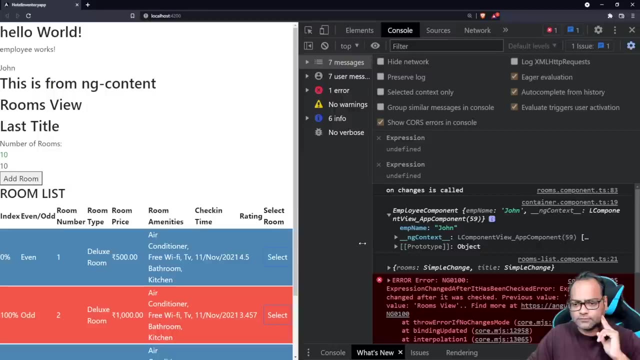 here. so we have to actually just go ahead and do whatever you want to do with this particular component or access this component here. so let's uh do consolelog, this is what employee right now and let's see our application. so here, um, let me just so you can see here, so you have access to uh line number ts. 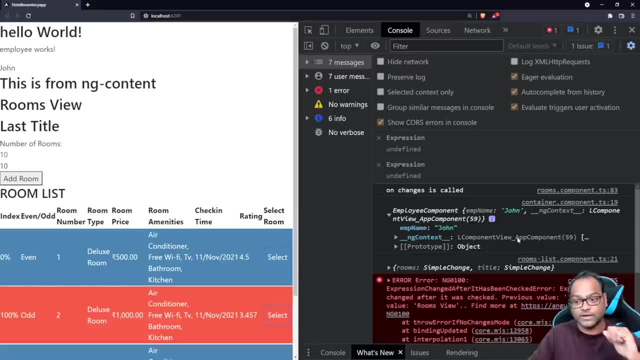 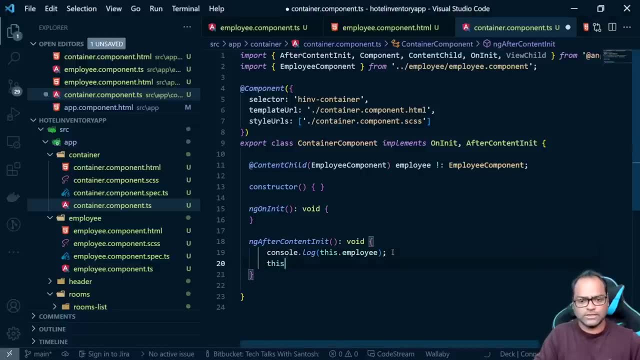 uh, you can see the line number here, so which says: okay, this is coming from container component. and then you have the emp name- access to emp name as well. now what i can do with this. so i can just uh, do something like i can change Telestart employee. 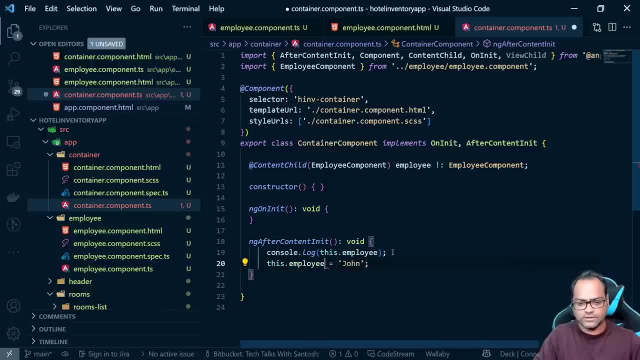 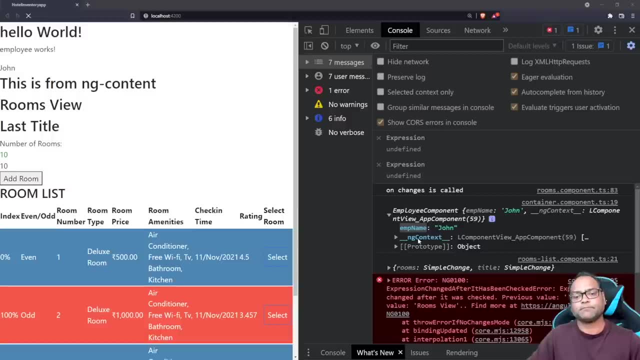 and i can just access the, let's say, dmp name becomes 2 from john and it will be changed here. so you have uh, the updated value available, so you can actually dynamically uh. so like i have updated value, uh in this鳥pnvenis, it knows this value. it enough kind of, and i can see it means to be rooted in this um and i think it could years. um, let me pull that in, is month64. 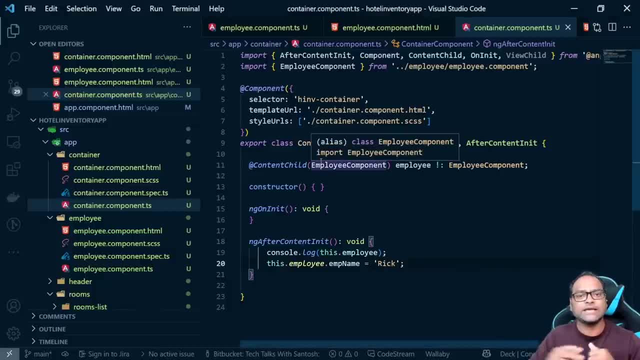 so i can just, uh, do something here. i can change this dot employee and i can just actually access the, let's say, dmp name goes to from john and it will be changed here so you have the updated value available. so you can actually dynamically- sorry, you can- actually access any component at runtime. 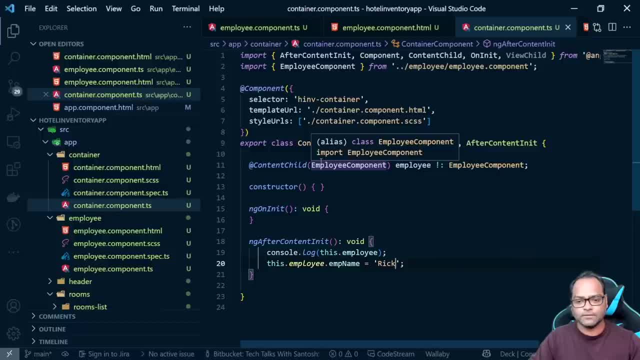 So it's not like something which is: you can access any component which is loaded via content or ng-content, Then you can access that component using content-child and then you can do whatever you want to do. So the preferred way is always, of course, 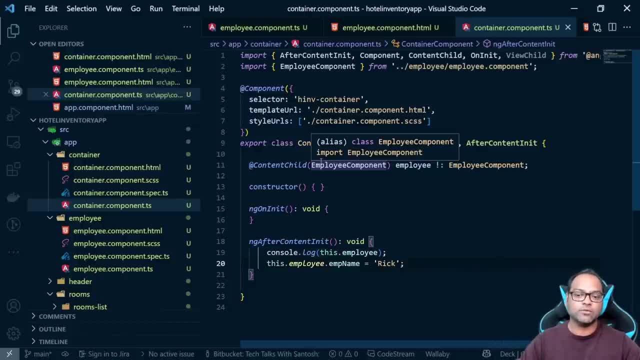 using input and output. you can make as much or you can. sorry, The preferred way is to use input and output, but in some cases this is really useful- view-child and view-children- where you don't have much control on your component. 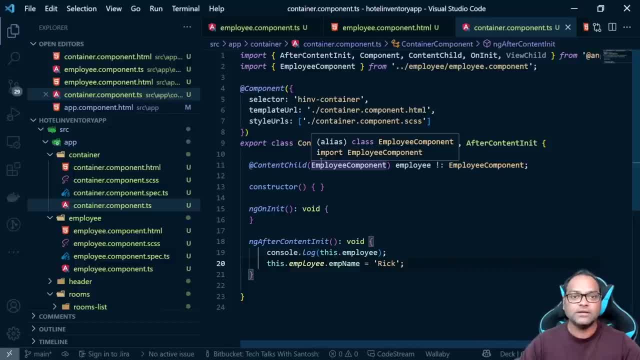 You want to access those components inside your TypeScript file, You want to create the instance at that particular time, and then you want to assign some data, or you want to actually bind some data or call some function which is available on another component. So these are the some use cases. 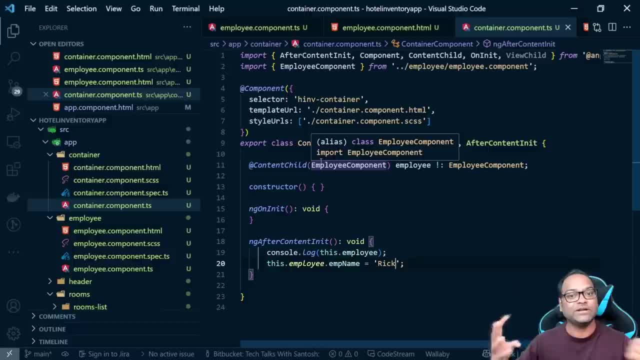 where these two are really useful, Of course, both having different purposes. right, We saw what view-child does and now we are talking about containers, So ng-content, remember this fact. So, in case you want to, you are not sure. 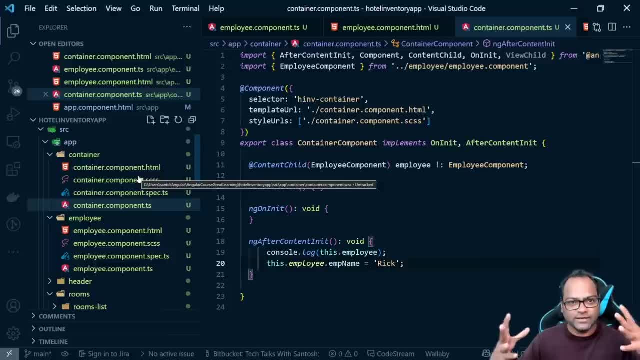 okay, what will go here? You just want to provide a container where I can replace any text in future, So you can actually add that inside the container, For example. one example which we can give is FAQs, right? So in case you have a lot of clients, 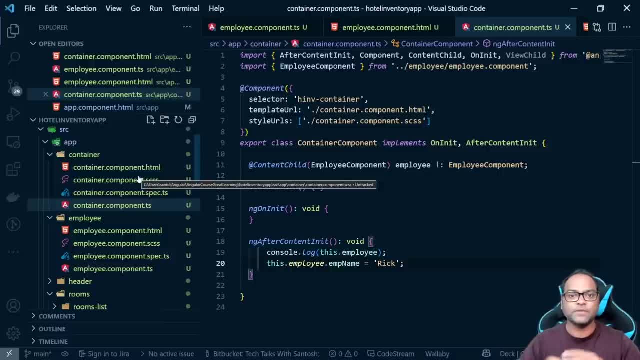 what you will be doing is, of course, the design will remain the same. Probably the only thing will change is content. So what you can do is you can create a container component, apply all the stylings you want to, and then just ask your designers. 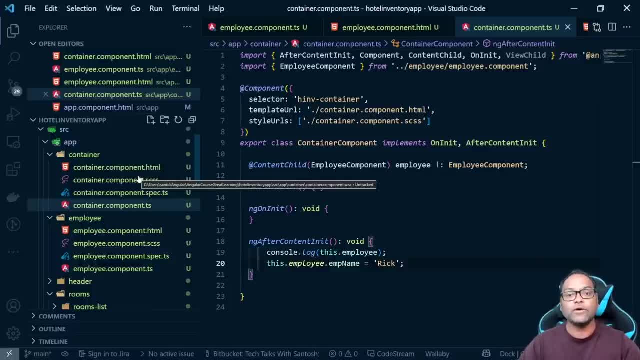 to actually write the content for you. that's it, Or whoever is responsible for the content. They can provide the content, that's it, And that saves your time, right. So let's move on. and now ng-after-content in it. 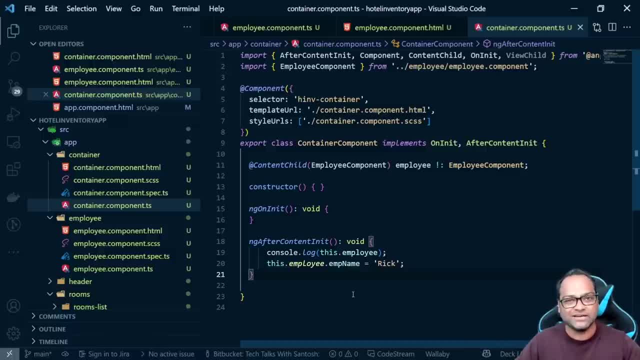 then there is a lifecycle called ng-after-content-checked. So in case you want to actually make sure something needs to be done once your, once, one time your change section has executed, you can use that, but probably rarely used, So you will not find many scenarios where that will be used. 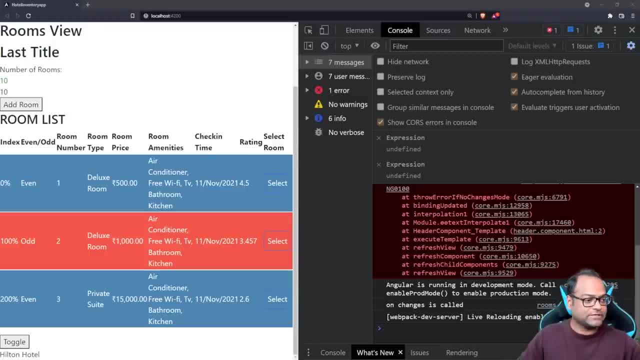 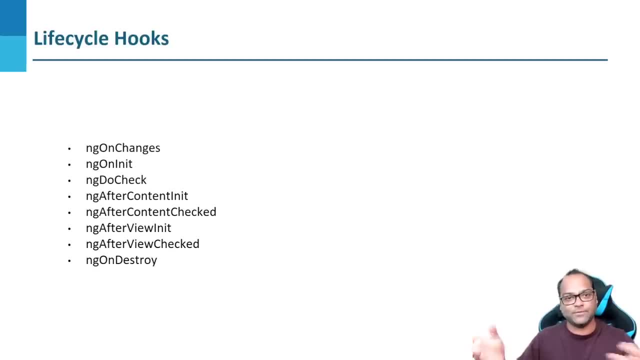 Which leaves us to our last lifecycle look, which is really important, because whenever something is created, it needs to be destroyed, of course. I mean everything. it's part of the life, right? So our component starts when it is initialized and when it is destroyed. at that moment, 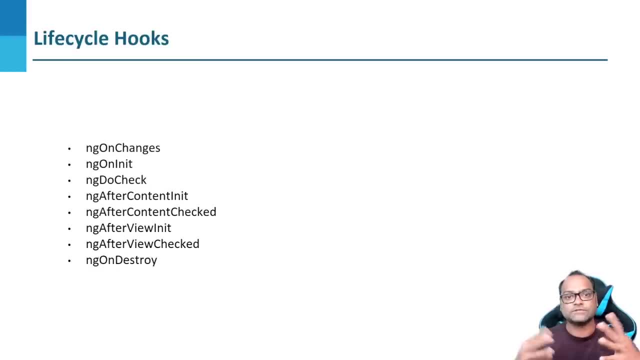 our last lifecycle- look which you can see at the bottom- is ng-on-destroyed, which on destroyed, I mean it itself says when I'm getting destroyed. So this is the event which will be called: when your component gets destroyed. But when does our component gets destroyed? 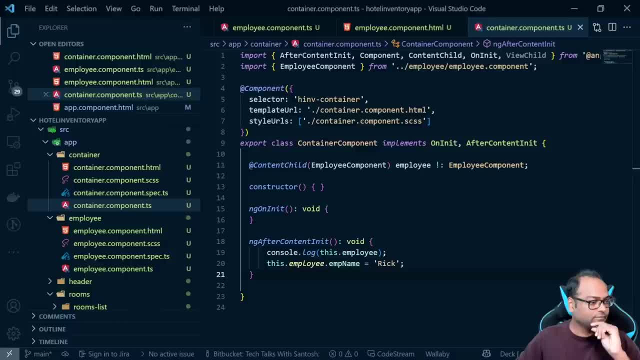 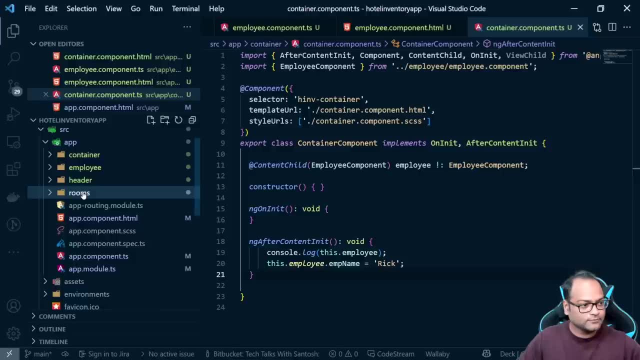 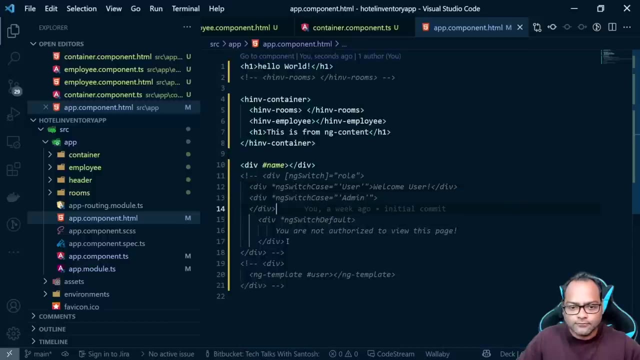 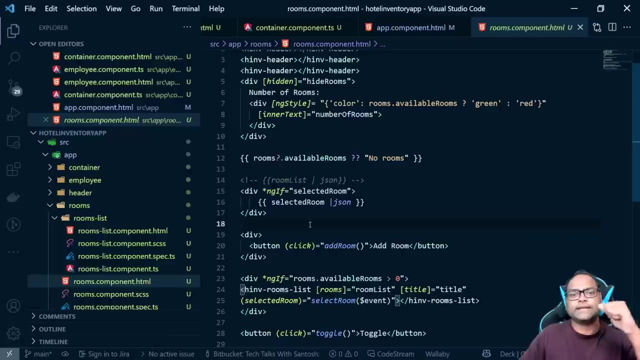 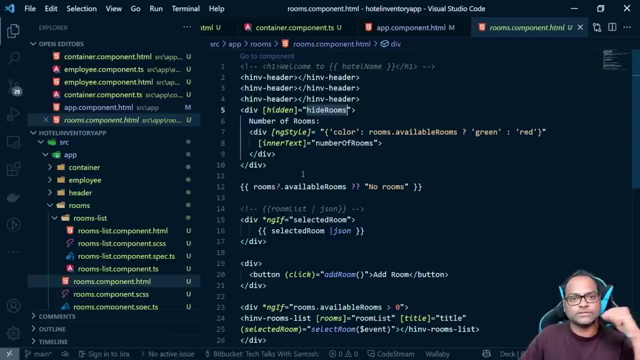 Very important question. Let's go ahead and figure that out. So here let's take an example of this. So remember, we had this hidden, right. So what I'm going to do is now I'm going to use ng-if and I'm going to use ng-on-destroyed on this. 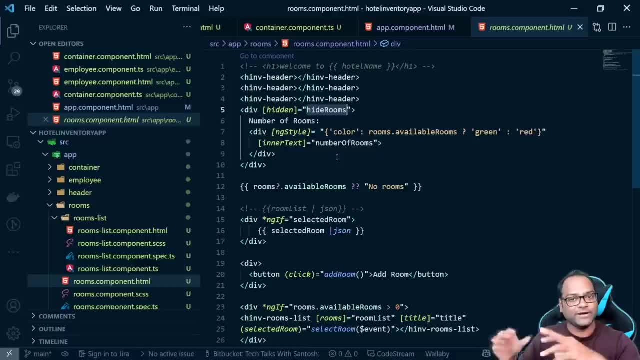 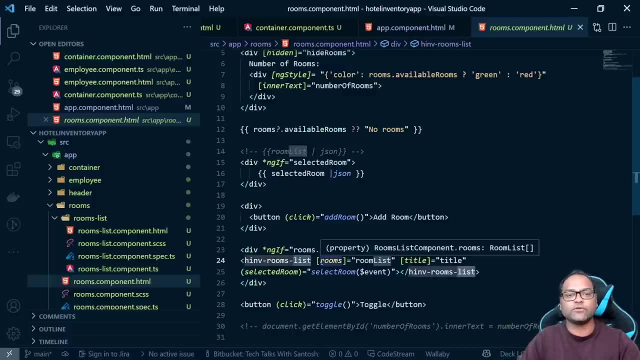 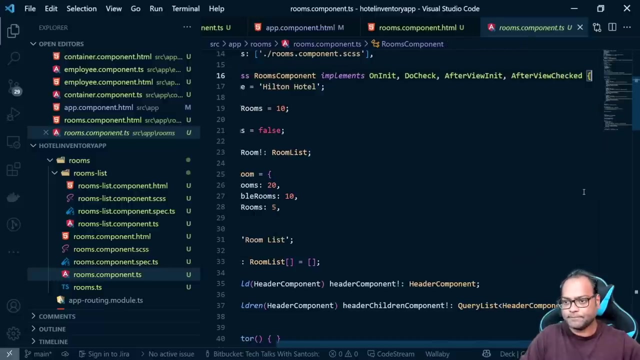 But what I will do is, whenever I click on hide rooms, we will hide the entire room list. Remember what ng-if does? It removes the component from the DOM. So let's use it here And let's implement. let's say, this is actually the instance in our project. 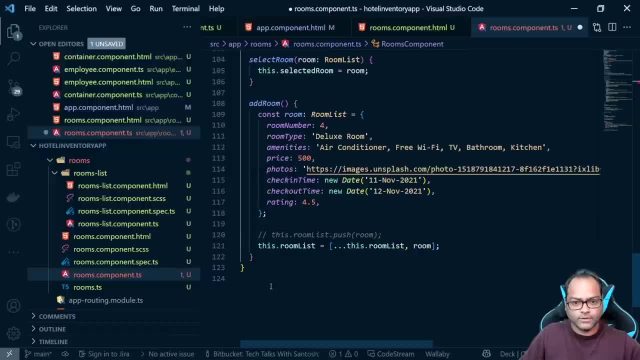 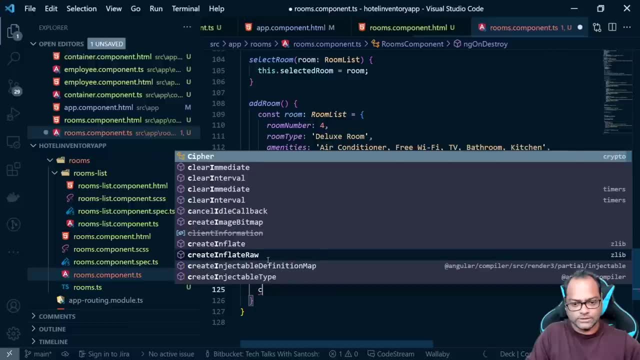 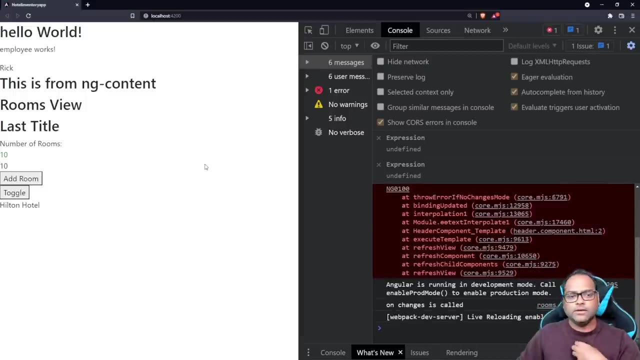 And I'm going to call it onKey And I'll return back to the engine And I'm going to say: this is a consolelog: OnDestroy is called. Let's go back to our code. So I'll remove, clear the console and let's click on toggle. 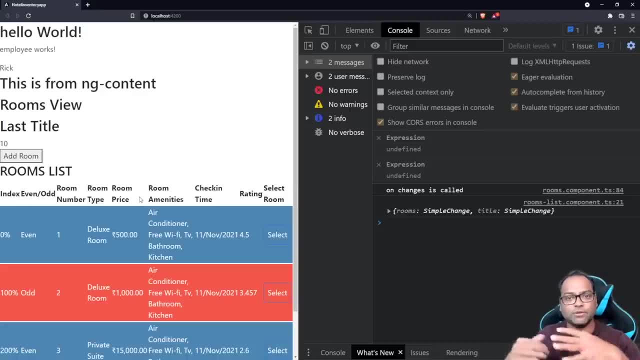 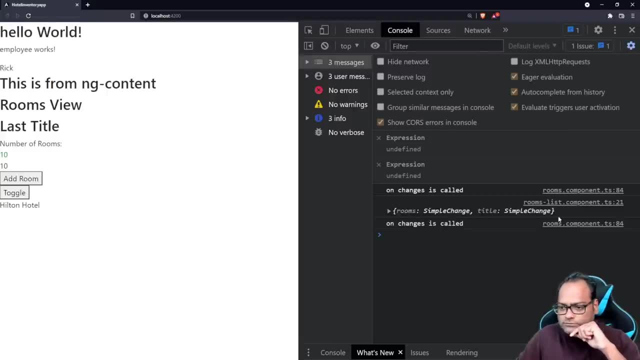 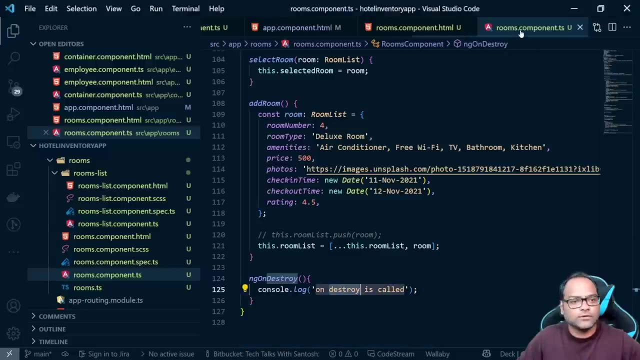 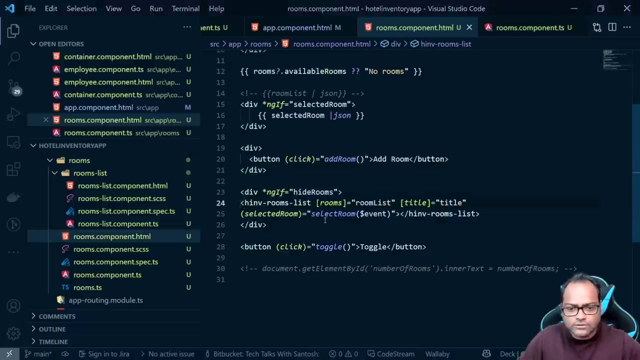 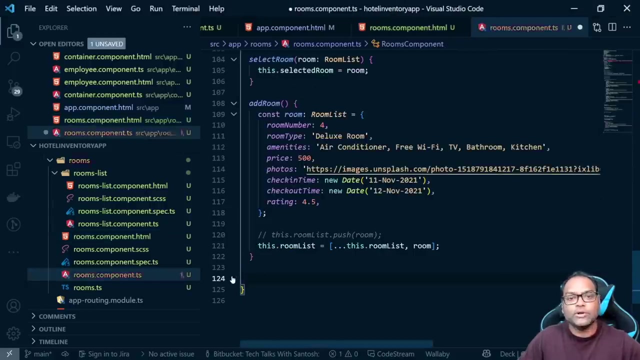 So you have your component back. So this is the first time your component is actually loaded. Let's click on toggle again. and I just implemented this on destroy at the wrong place, because the component which is getting destroyed is not this one, It is the rooms list component. 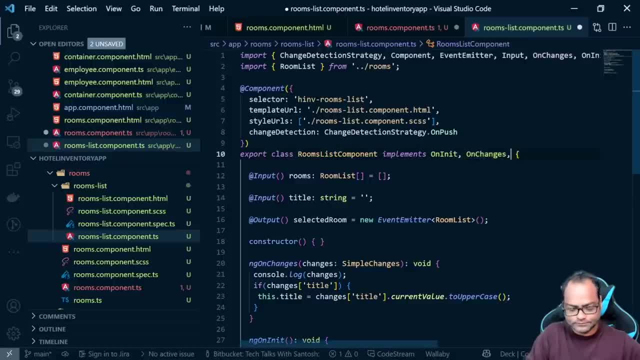 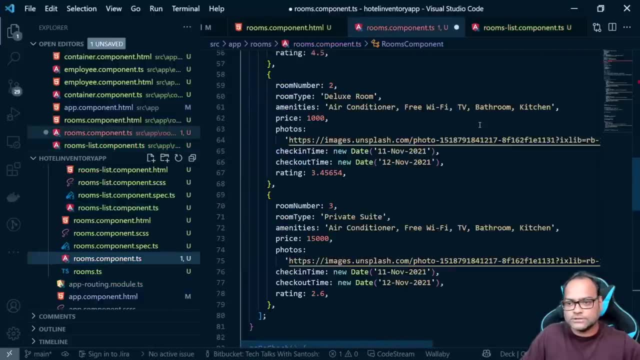 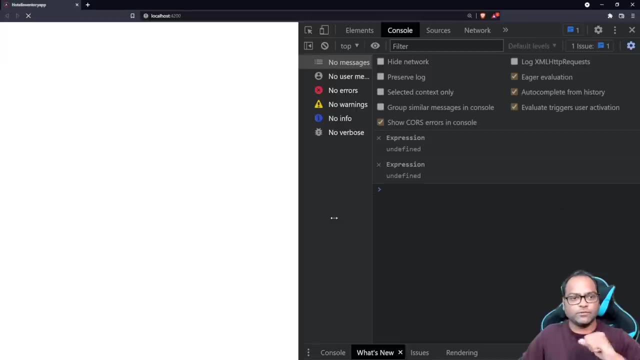 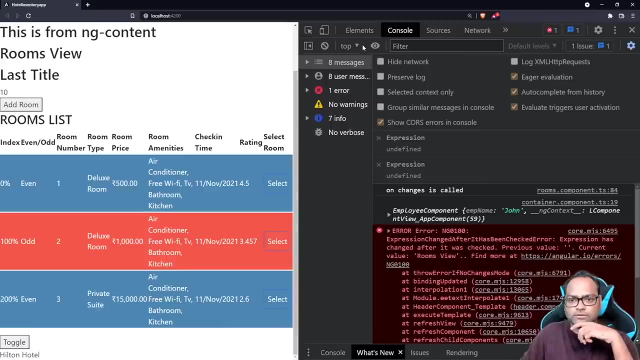 So this, and we'll just remove the on destroy from here, because otherwise it will give us an error that we have not implemented the interfaces properly. Let's see. So you, we have this toggle button, Now the component is loaded and let's clear the console and click on toggle again. 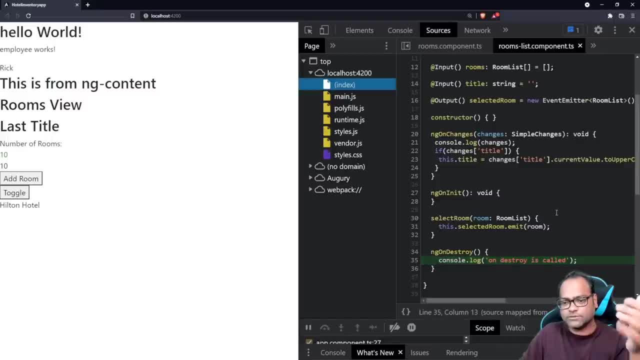 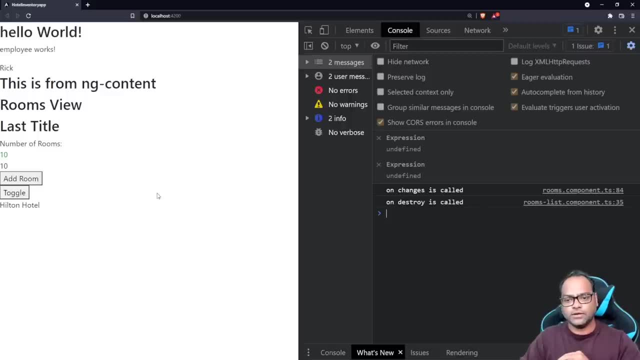 And you can see now it says: on destroy is called And rooms list component. just to clear that. okay, this is the correct line where this code is available. So what is happening here? Why on destroy is getting called. So remember so. whenever the DOM element gets removed, sorry, whenever a component gets. 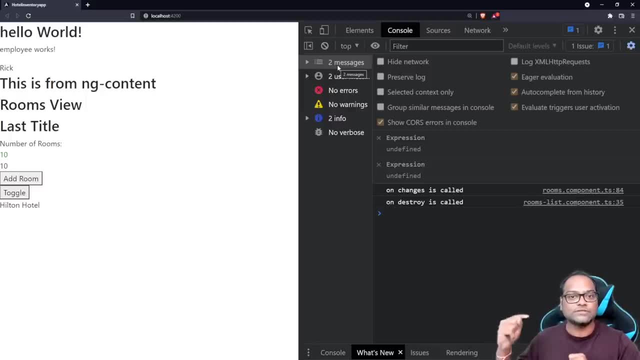 removed from your DOM. at that moment, the components on destroy lifecycle event will be called. Now what you can achieve using ng on destroy: So it's getting destroyed, So it should be okay. I mean it's okay, It's getting destroyed. 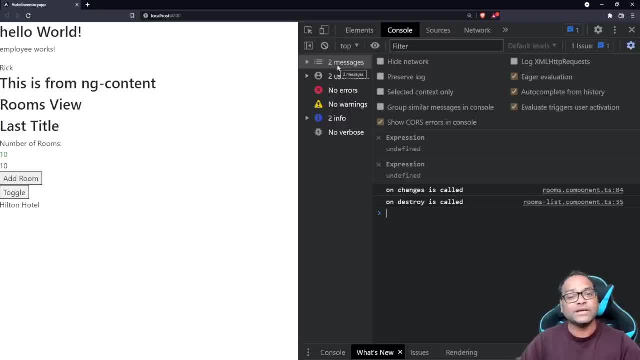 But it's really useful in case you have some memory consuming code and you want to free the memory. This is the code, This is the lifecycle. look where you can actually do that. Now, what is the scenario for Angular? So in Angular, we will be using something called subscription in upcoming sessions. 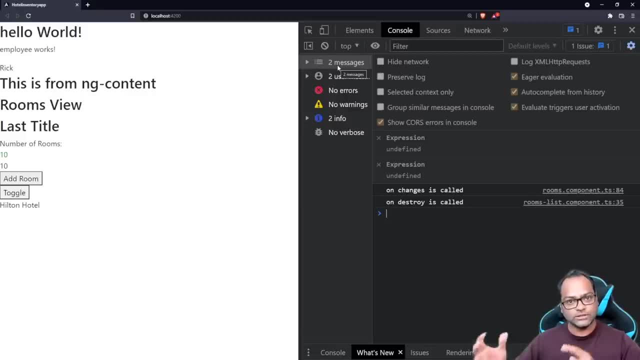 in upcoming videos And using those subscription, you can actually subscribe to some data. Now, once you subscribe to that data, That's that subscription become active. So somewhere you have to actually unsubscribe to those. That's where ng on destroy comes into the picture, or you want to actually probably 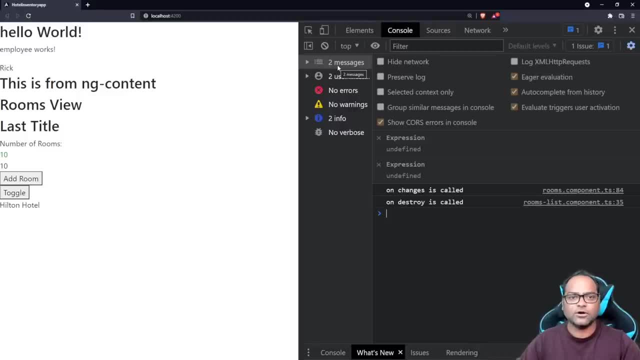 let's say, reset some data or do some logic whenever your component is getting destroyed. You can go ahead and do that inside ng on destroy. For example, let's say you want to remove something from local storage or session storage whenever a component is getting destroyed. 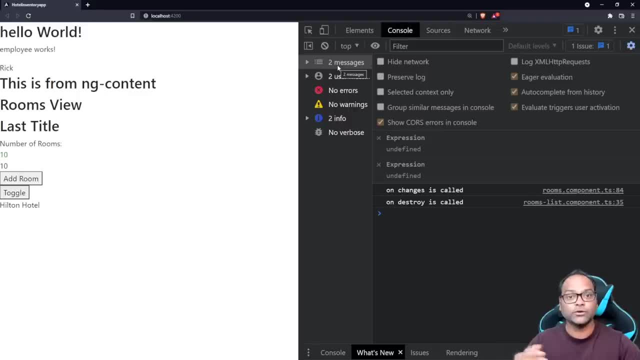 Yes, That's the lifecycle book where you can book into and call those code to clear your cache, clear your storage. Those are the things which can be done here, But most of the time you will be using this lifecycle. look to unsubscribe to the data. 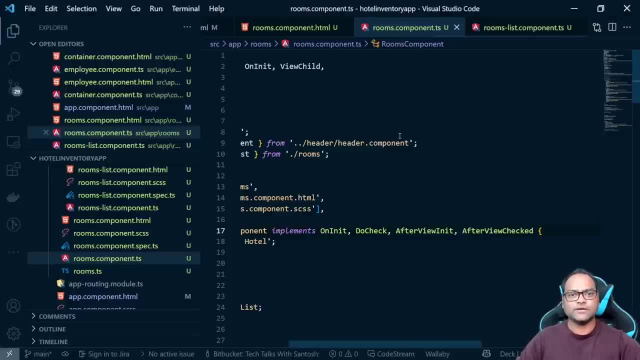 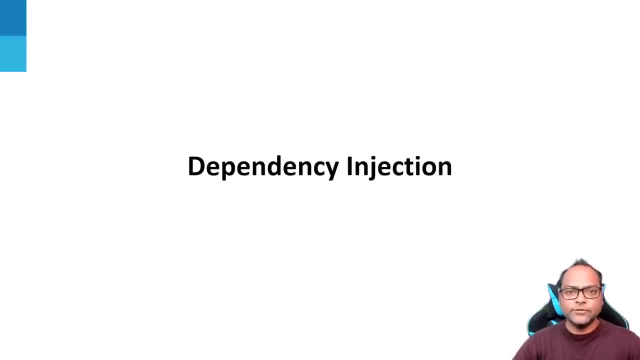 in future. So this is it about lifecycle looks. Now let's move on to the next topic In this video. we are going to talk about dependency injection. So we will talk about dependency injection. We will talk about what is dependency injection and we will see what is DI providers. 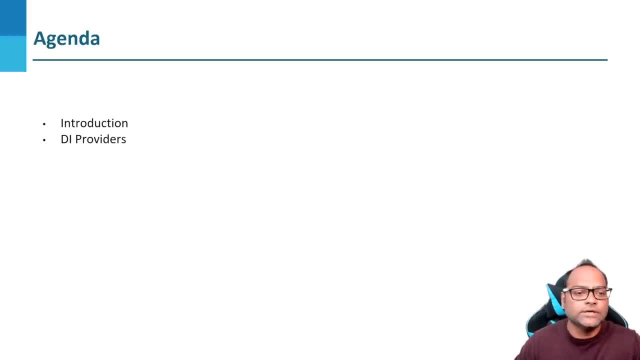 So DI stands for dependency injection, make sure. So let's go ahead and talk about dependency injection. So dependency, in case you are coming from some other technologies you may have already used it, For example, NET and Java uses dependency injection a lot. 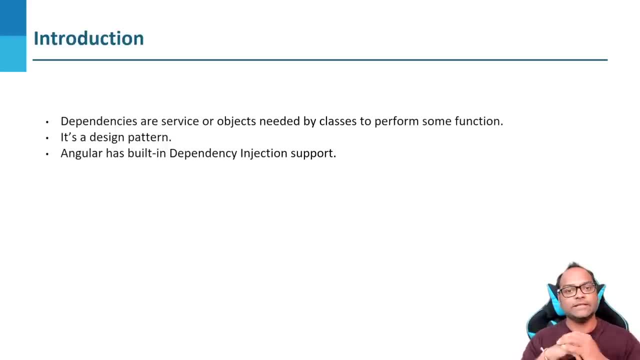 But in case you are not aware, that's absolutely fine. So what is a dependency here? So in Angular, dependency can be a service. So in Angular dependency can be a service. So in Angular, a dependency can be a class or an object which you can access, or you. 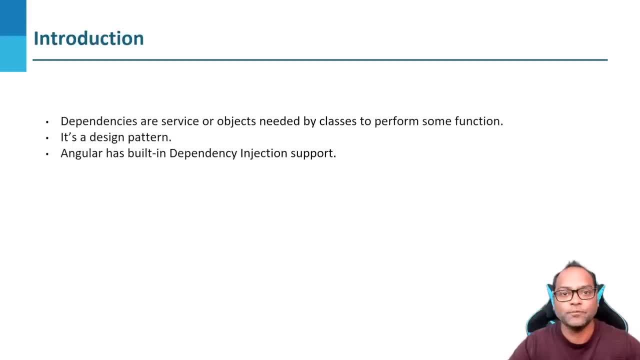 can inject inside a component or inside a service, wherever you want to. It's actually a design pattern which is, as I said, widely used in other technologies- NET, Java- they use it a lot- And in other technologies. 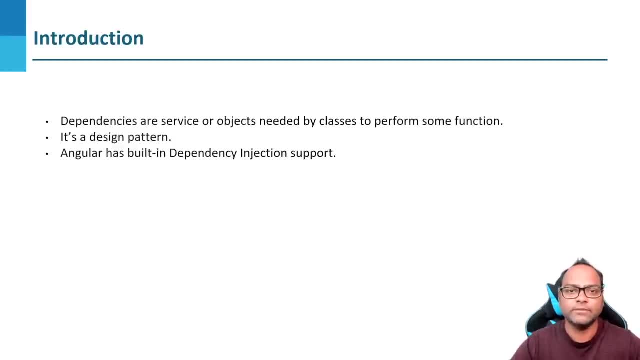 So you have to actually go ahead and do some configuration to actually achieve dependency injection. But Angular has the dependency injection built in And this is one of the- I would say one- fun. So dependency injection is one of the features which actually makes Angular what it is. 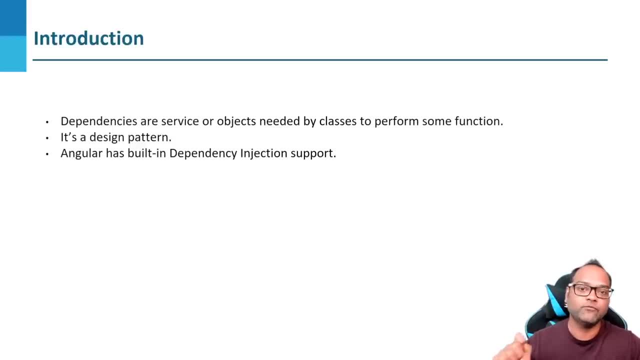 It makes Angular really better, because this is one functionality, or you can say one feature, which is not available with other frameworks, And it is really powerful. So we'll, of course, go ahead and see what we can achieve using dependency injection. As you said, there are multiple types of providers. 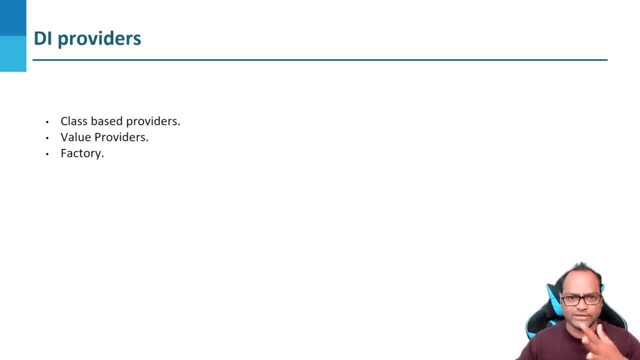 So you have class-based providers, then you have value providers and we have factories. We'll talk about those. what are those? and we can also, before we actually go ahead and talk about other DI providers, we'll start with class-based providers. 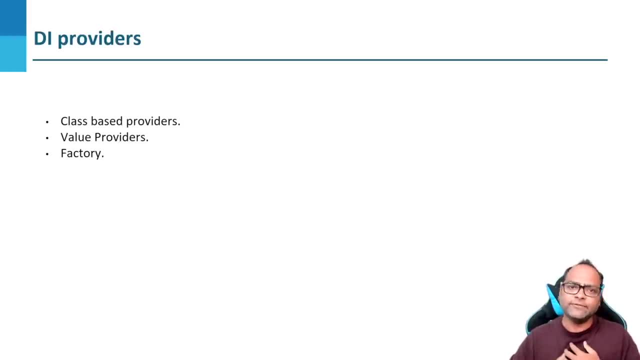 So we'll start with class-based provider, then we'll see value provider And we will see factory as well. So here let's go ahead and see how you can create and consume a service. We'll also talk about what service does. 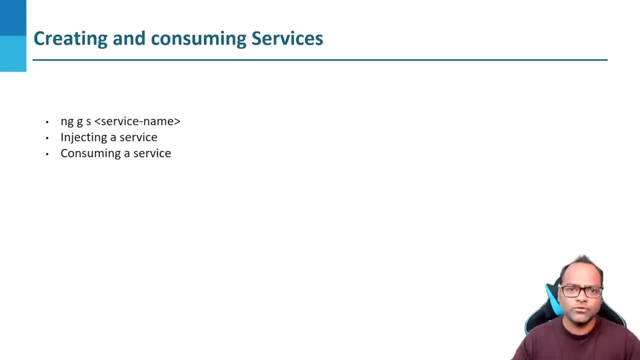 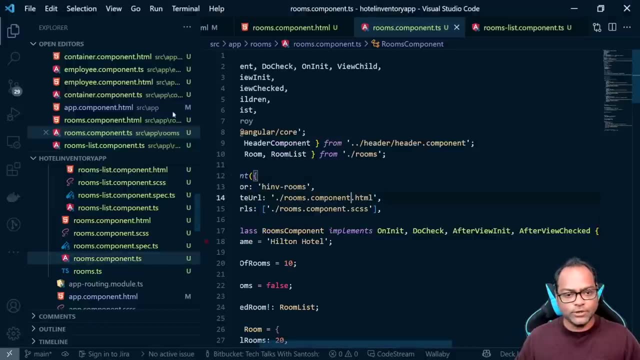 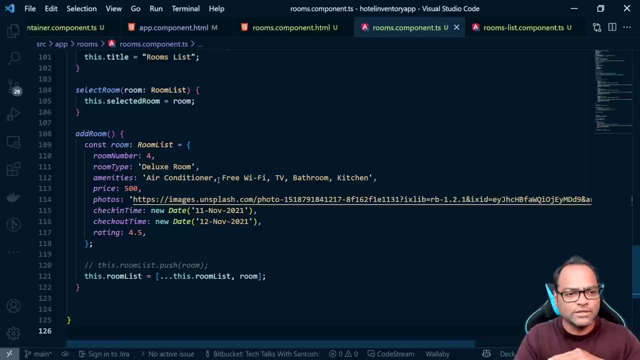 Because that's important: right Before you go ahead and use something, you have to be aware why it is used. So here, rooms-componentts, let's go back to this component. So if we see, the number of lines of code in my rooms component is already raised around. 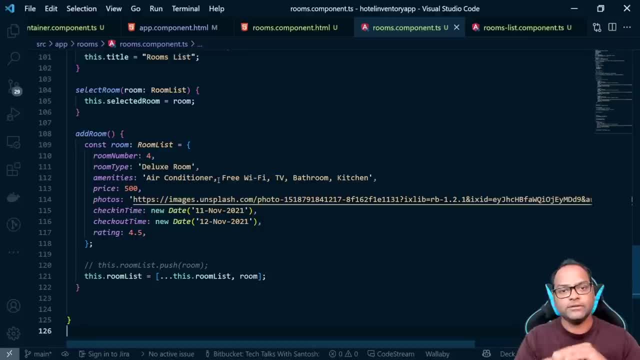 126.. I mean including, But yeah, I mean more than 100 lines of code And some of the code may be reusable right. So not right now but of course in longer term- some of the code which we have written. 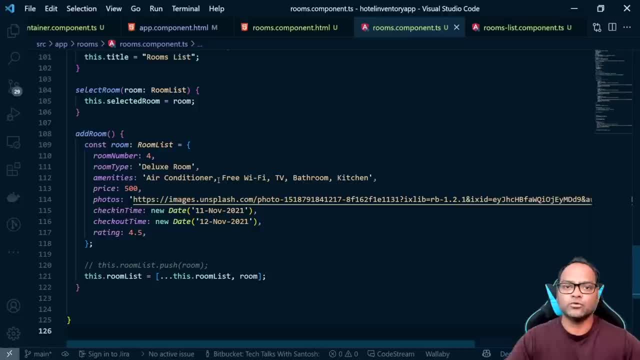 inside room component can be reusable. So what we can do, Of course, what we can do, is we can create something reusable and we can move this code somewhere. What is that somewhere? So that somewhere is service. So what we can do is we can create a service. 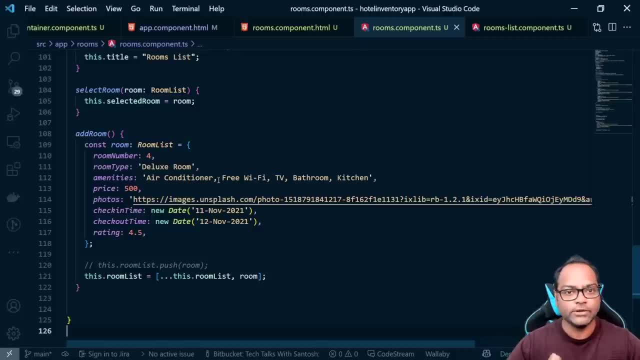 We can move all reusable code in that particular service. Generally, what you try to do is keep the code minimum inside your component and try to split that code into multiple services. I mean services is something where you will be writing your business logic. 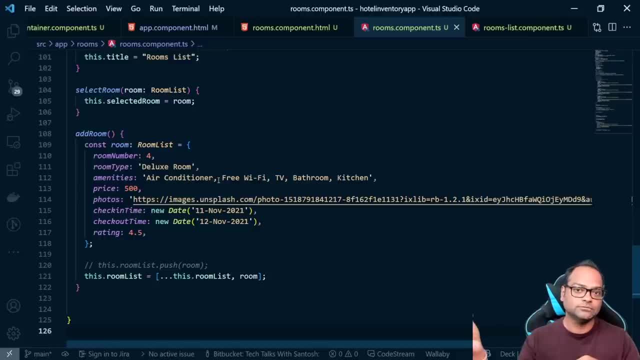 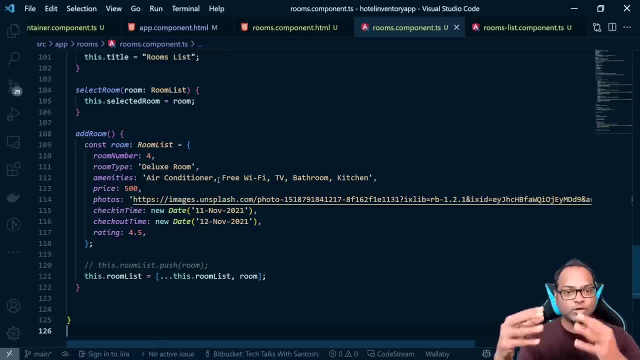 What is this? What is this? This is what it's supposed to do. For example, it's possible that you may do multiple things inside a component. For example, you can have a dashboard where you are accessing the data from. let's say, 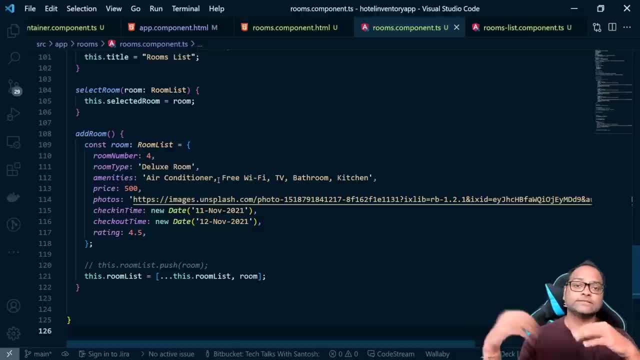 employees. you are accessing the data room data. you are accessing the booking data. So what you will do- write all the code inside your component? The answer is no, Of course. what you can do is you can create multiple services based on what each service 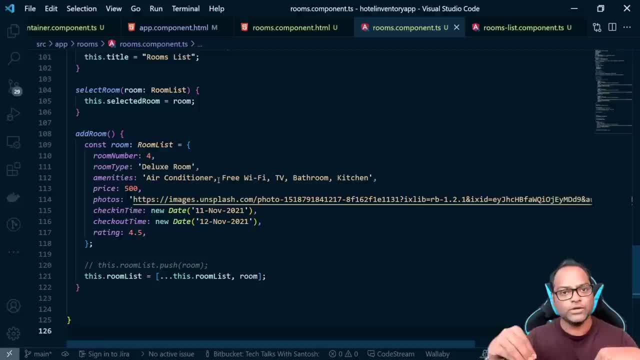 is supposed to do, For example, each service, One service for rooms, One service for booking, One service for work, For example, one service for food for employee, and then i can just use all those services inside the component and the uh, the. 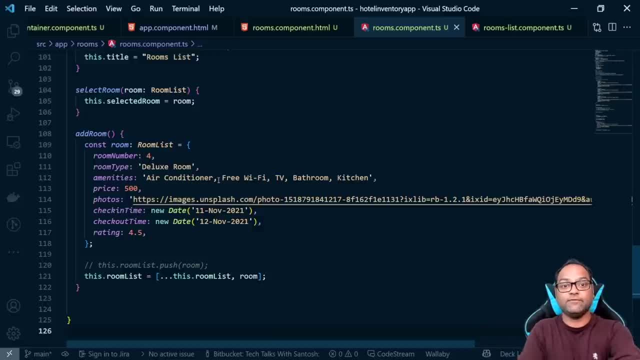 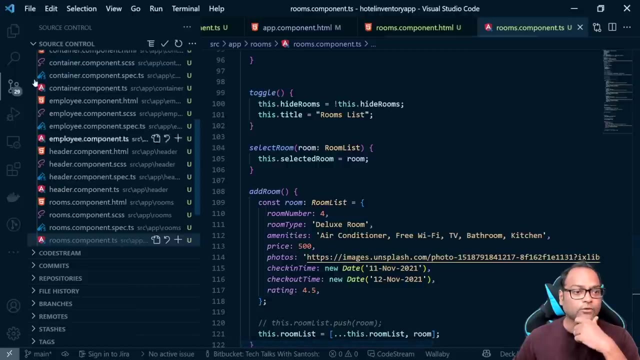 advantage is i can actually go ahead and use that service anywhere i want to and i don't have to duplicate the code. so let's see how we can actually do uh, or start creating a service and split the logic in this example. so what we'll do is we'll create a service for rooms. now for creating the. 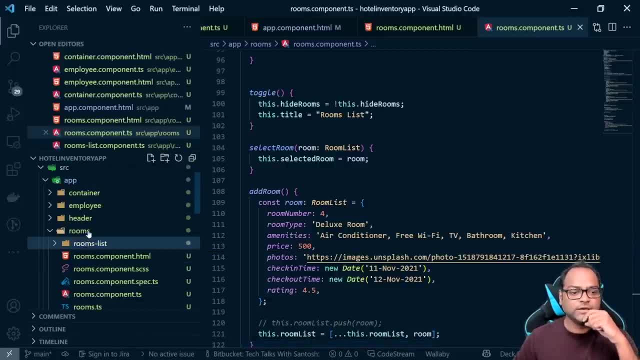 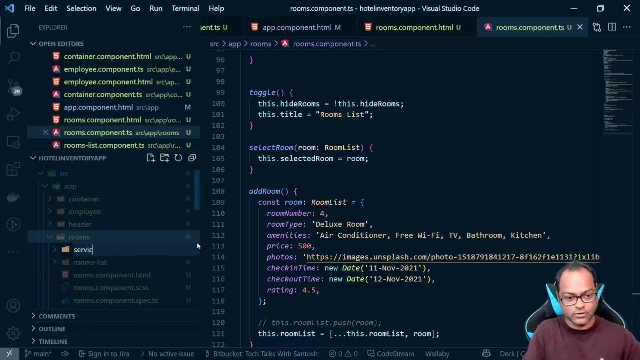 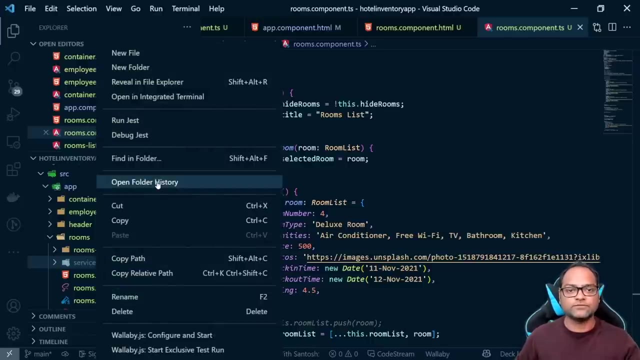 services. it's up to you what folder structure you follow generally. uh, what i do? i keep a folder called service or services and i create my all services here. for example, any service related to rooms goes into this folder. similarly, i mean, if i have to create a new service for employee, i 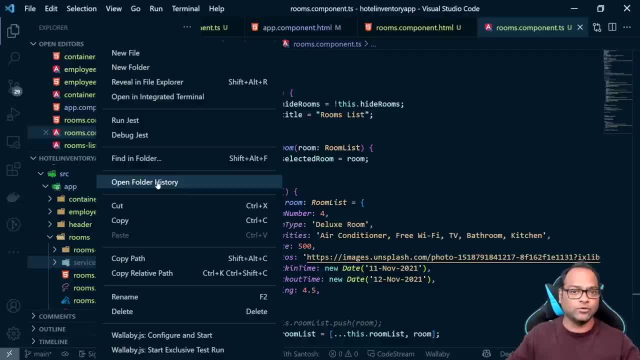 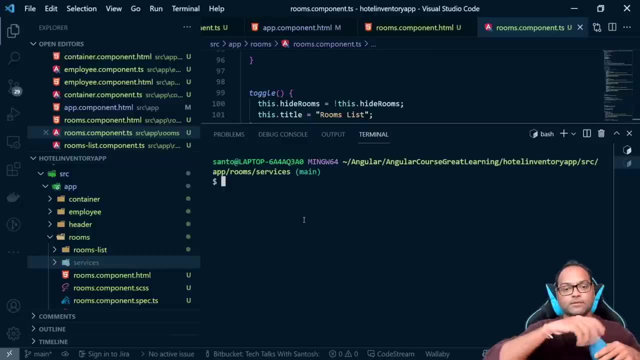 create a services folder in employee and then move all the code base or add all the logic there. so let's, let's go ahead and create our service. so we won't be doing it manually. we will be using angular cli so you can type ng g, generate as service and the name of your service. so 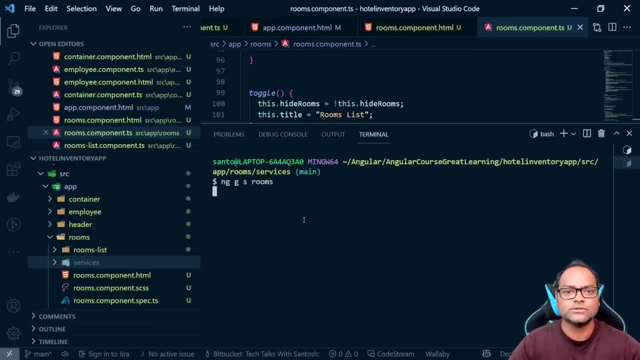 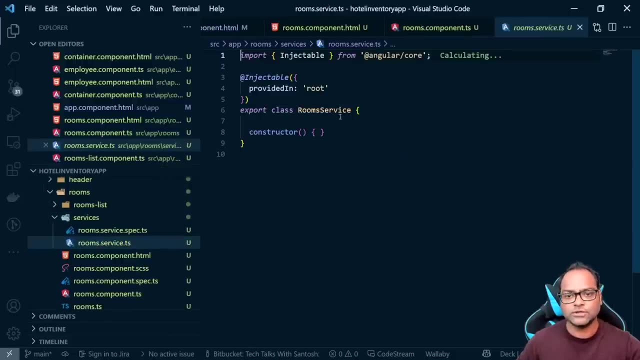 here. i want to create a service for rooms, so i'll say okay, rooms, so my new file. you will be created inside the services folder and here it is. so you have rooms or room service, uh, class created so you can see, okay, it has a, it has a class, and then provided in root. 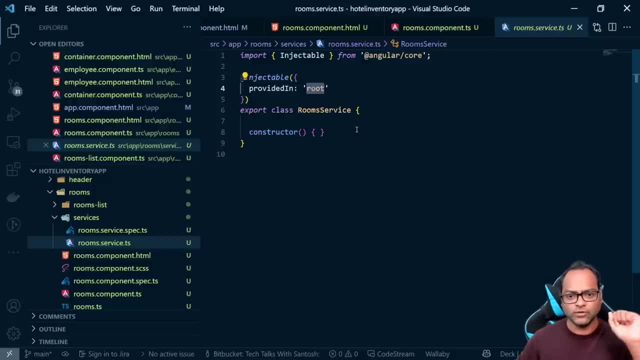 what is this provided in root? we will discuss about it. let's ignore it as of right now, and what we will do here is we will move some logic from my rooms component to here and then we will use this service rather than actually writing that code into room service. 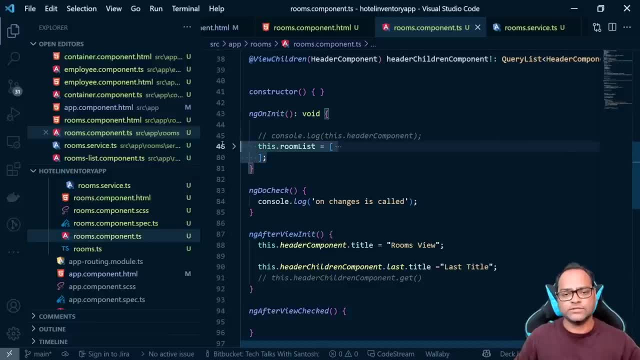 let's see first this data. right, so we have actually this data which is coming, for example, in future, what we will do is we will get this data from our back end or from some api. so generally the retrieval of any data should go into a service. so here i can create. 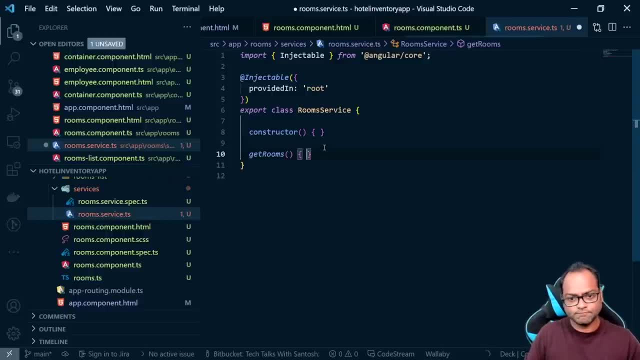 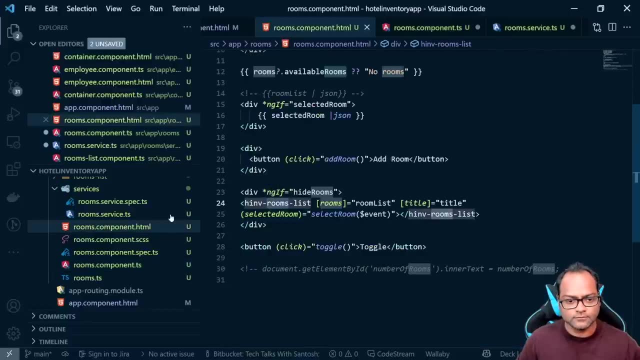 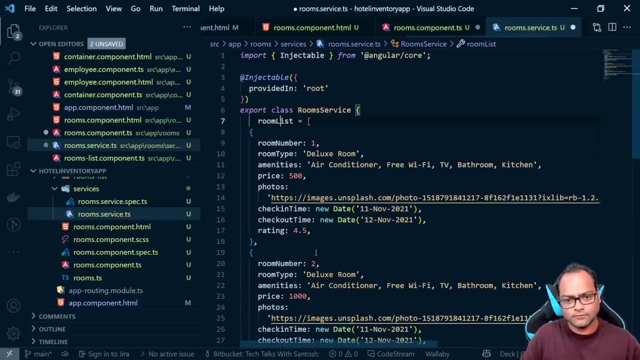 a method. i can say this is get rooms. so here i can create a method. i can say this is get rooms. so here i can create a method i can say this is get rooms, so snacks, so so i'll say this is this room's list. so i'll say this is this room's list. 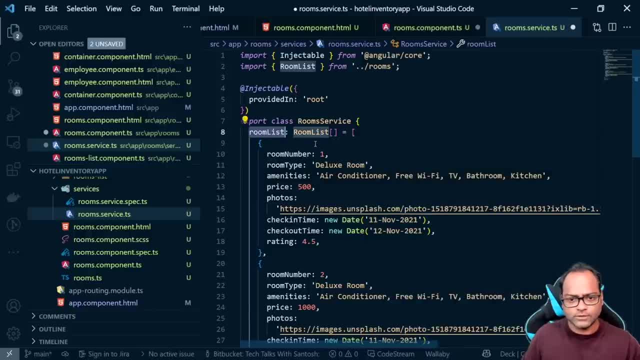 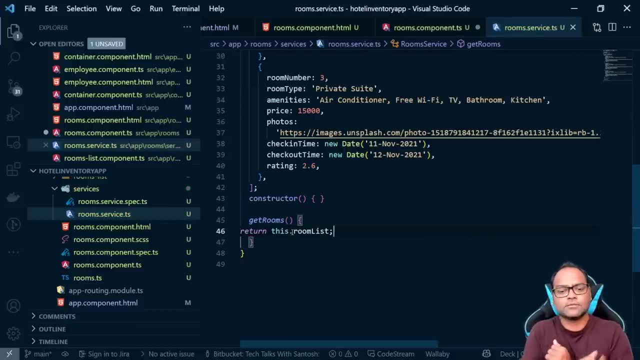 sorry, and then i'll just return this dot home list. so sorry, yeah, i'm not able to extra t here. i think that we have it correct here, but okay, oh, i guess so. So nothing extraordinary right now because we don't have the APIs. we just want to understand. 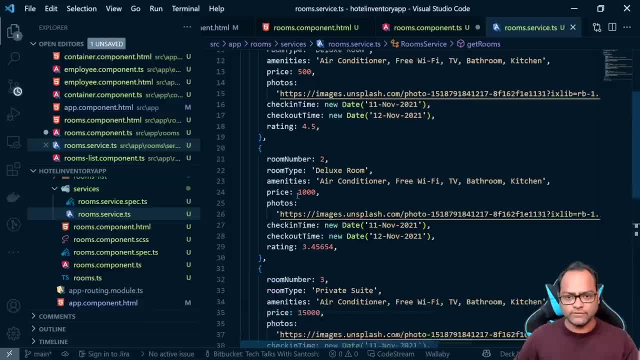 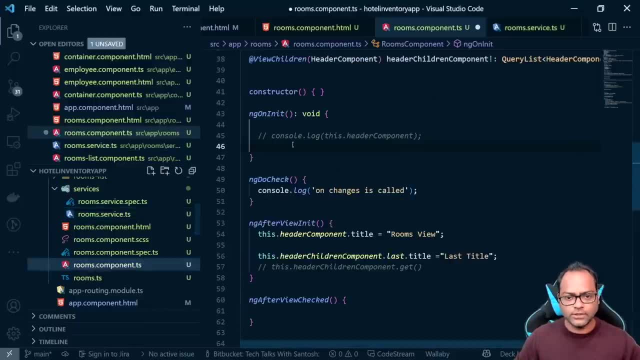 how services works. So we got the rooms data, which is now part of my service, And rather than actually doing or getting all the data- I mean inside the component- what we have done is we have moved that logic into a service. 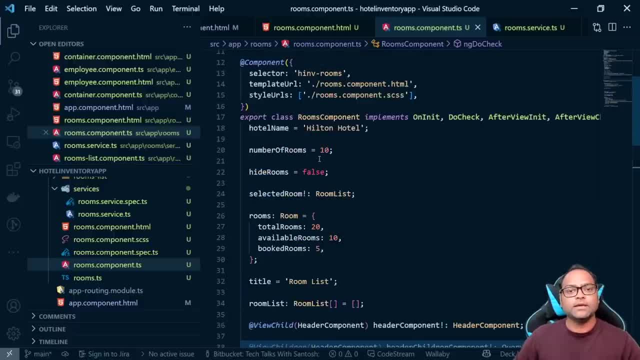 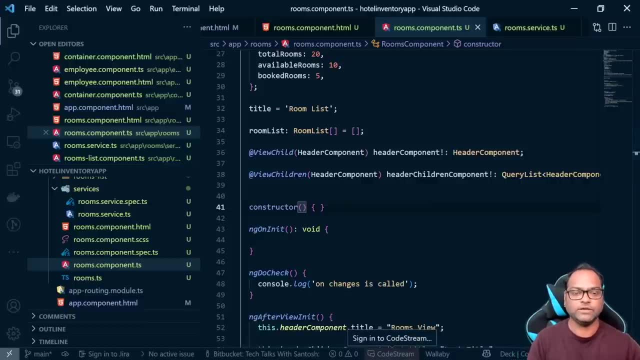 Now let's see how to use that particular service. As we said in Angular, we are going to use dependency injection. So what is a dependency injection? It's a design pattern. of course, we said it's a design pattern, but what it does? 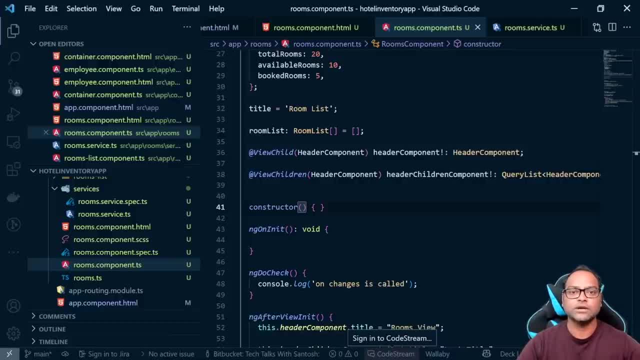 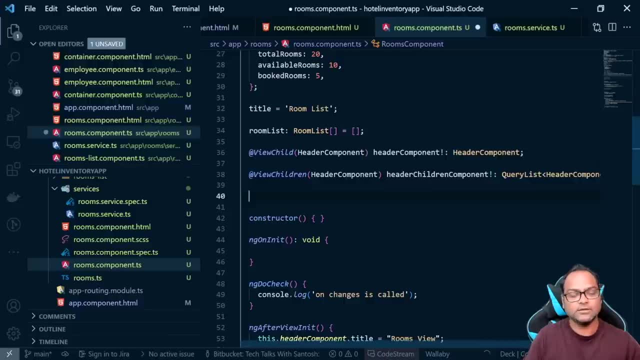 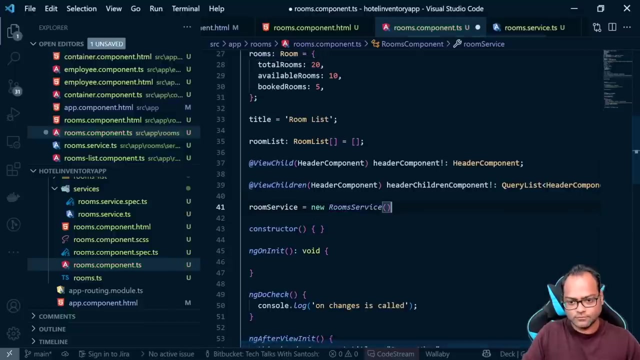 So using dependency injection approach. the dependency injection approach says you should not create an instance directly. So, in general, if I have to create an instance of class, this is something which we'll do. We'll say: okay, This is a room service which is type of, is equal to new room. 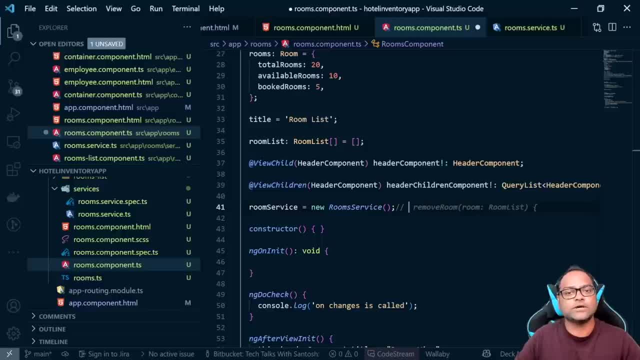 So this is how you will create a new instance of a class. But when we say we need to use dependency injection, this is something which you should not. So this is how you will create a new instance of a class. So this is how you will create a new instance of a class. 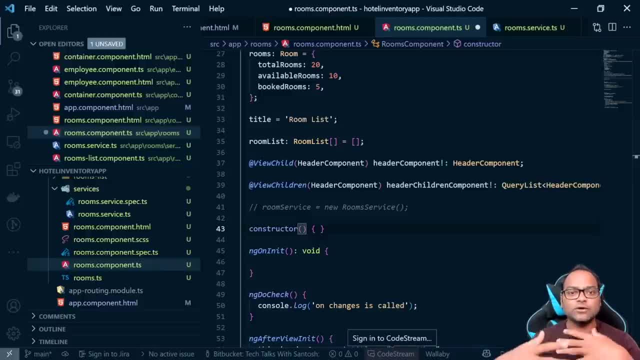 rather than creating the instance manually, we need to rely on the dependency injection which is already provided, built in by angular. we don't have to do anything else. so let's see how we can do that. so here i can inject a service. i can inject anything i can. 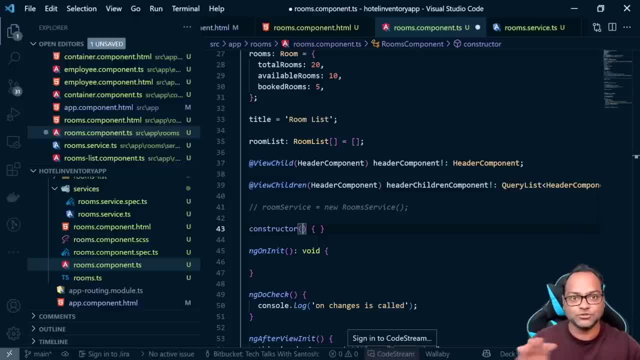 inject a class. i mean, even you can inject a component, which you should not do until unless you think that's the last approach possible, which i think, which i don't think. so i have seen some developers doing that, but that's an endивать and i would say: should not inject a component. 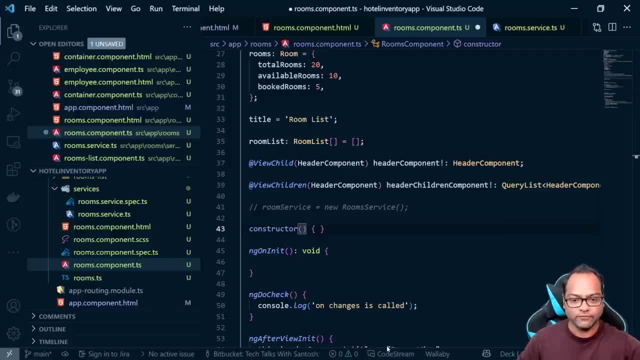 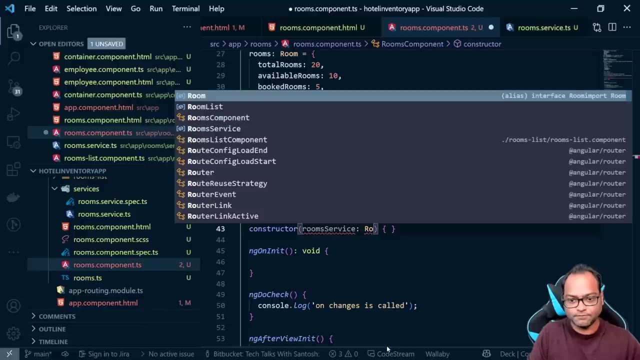 so here we have created a service and now we want to use this particular service inside our component. so this is this is how you will be doing. so you will say rooms, i mean the variable name service, which is type of rooms service. now, once you do this, 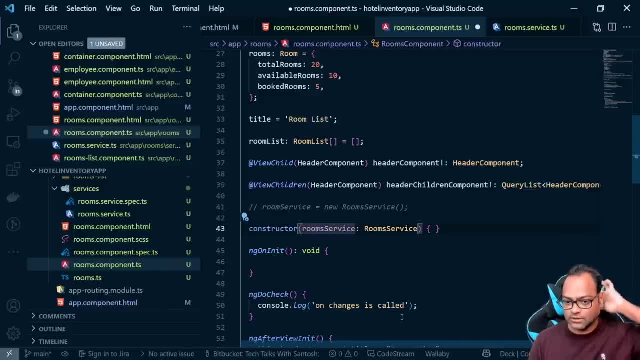 we have to also proppent, provide the access modifiers. Now this is where lot of developers get confused whether we should get it, get, take it public or private. I would say always make it private. The thing is, if I make this particular service public, it can be accessed on the template, which is again an anti-pattern. 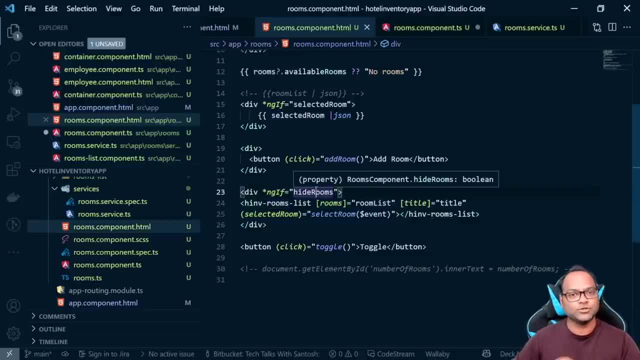 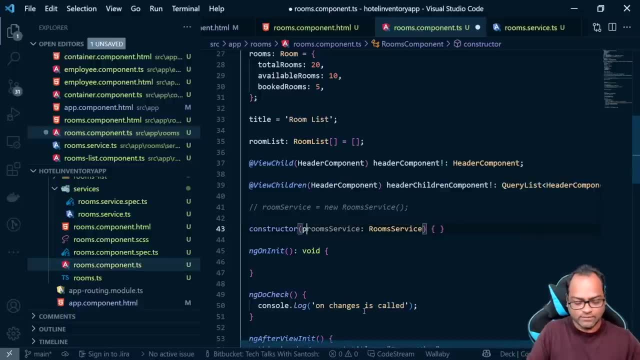 lot of developers does. it should not access services directly from your template. Try to avoid it. So what I can do is I can mark this as private. It means, okay, I am limiting this particular service to my template or, sorry, to my TypeScript file itself, not anything else. So it 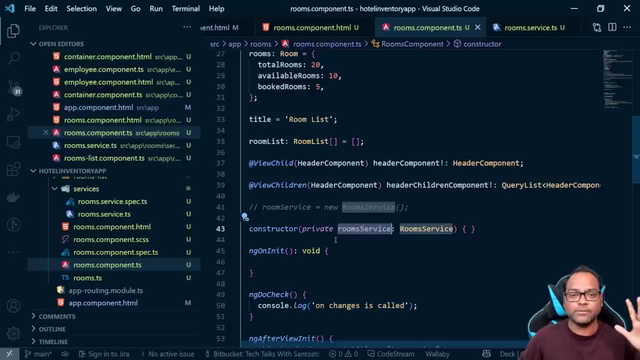 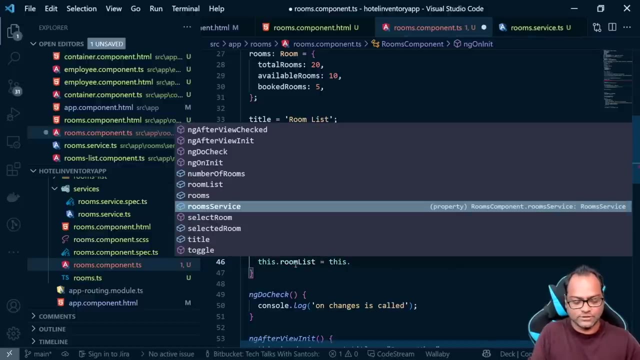 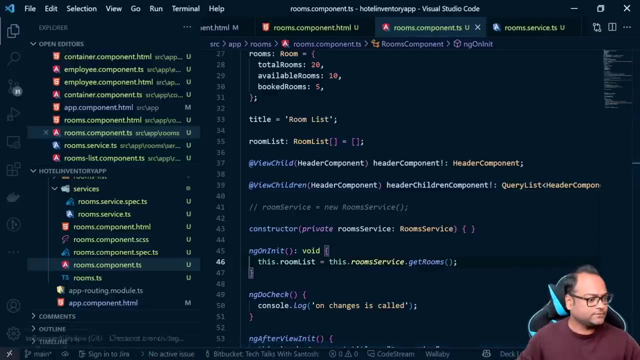 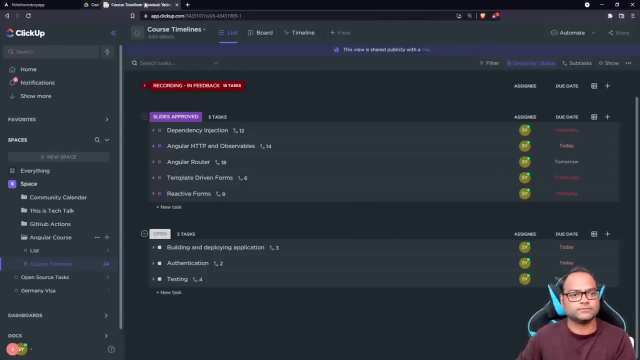 will. the instance will not leak onto my HTML or my template Now to get the data I can. what we can do is we can say this dos rooms list is equals to. now we have to get it from service. So we'll say this: dot rooms, service, dot get rooms, and let's go ahead and see the output. So let's go ahead and. 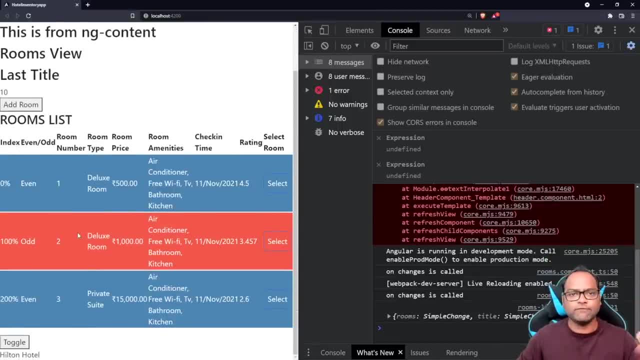 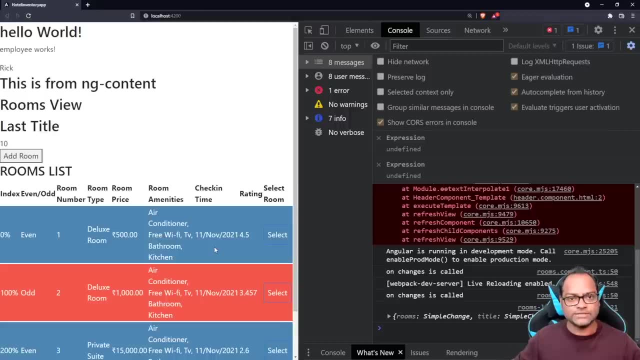 see the output. So here of course we have to click on toggle and you have your data back. The only thing, only difference is now this data is coming from your service, not from component itself. So component doesn't know how to get the data Generally. your component should not know how to get the data or how to 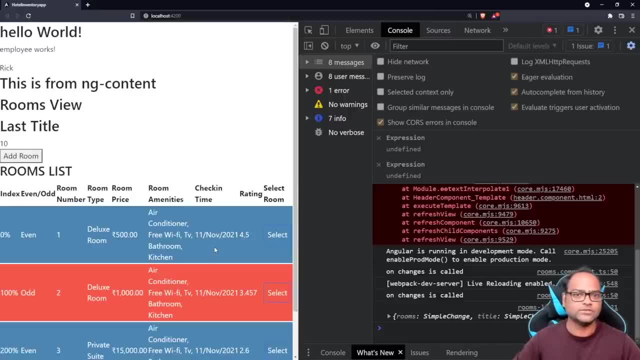 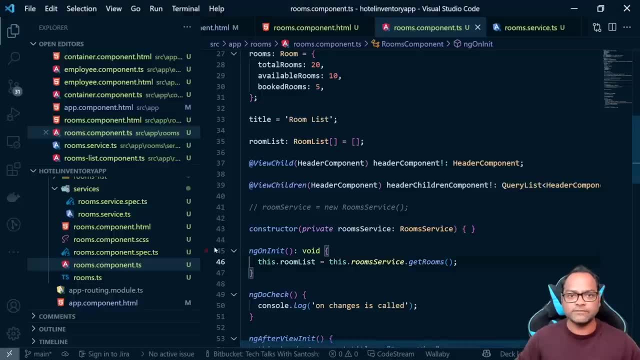 add the data or how to even do any business logic. That should not be the responsibility of your component. That should go into a service. So what? what is a service? a reusable class where you can actually put some business logic and then you can just access those inside your component? 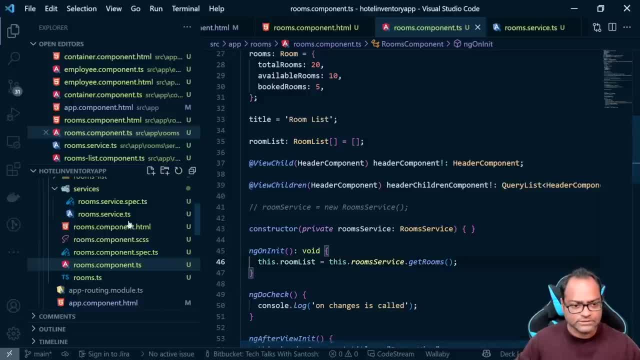 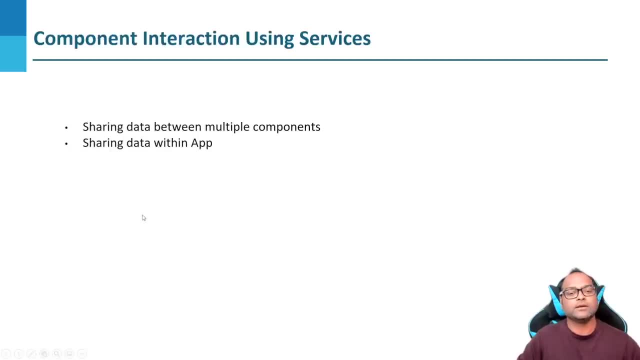 and this. this is how you will create a service. So let's go ahead and move on. You can also achieve component interaction using service. So, in case you want to pass the data between two components, you can do that using service. A better example, which we'll see, is when 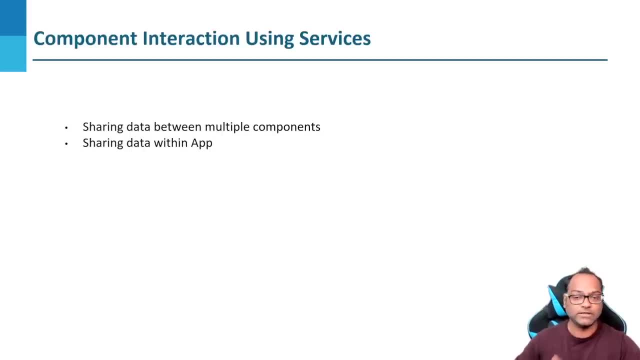 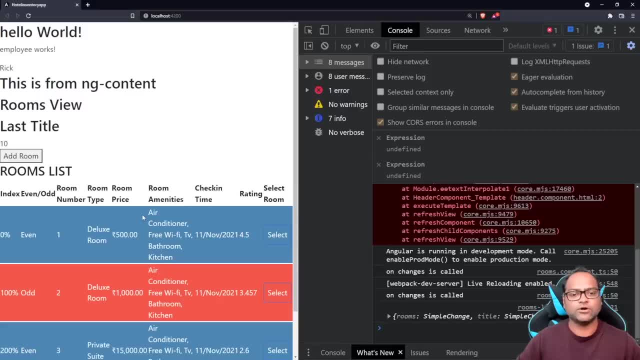 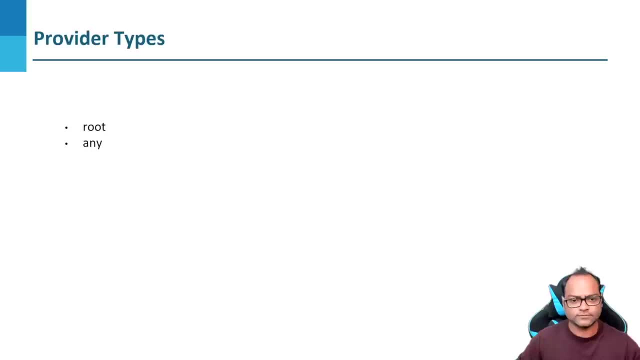 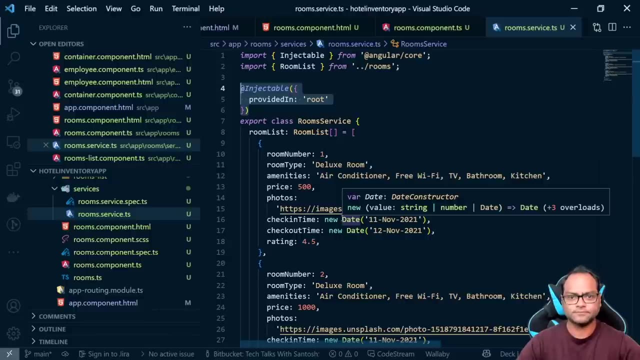 now we have to actually talk about let's, let's go into a little bit more detail into the services. So, provided we have root and you have two more, you have a root any, and there is one called platform, which is which is not used, which is in. 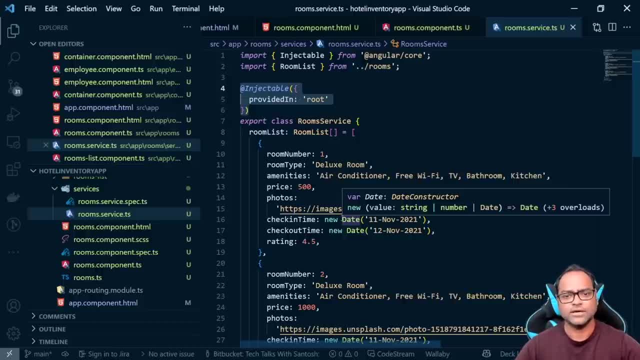 get which gets internally used by the router service uh. as of now, there is no like concrete example which is available for using provide provided in uh platform. in case there's something comes up, we will add a new video, but right now we have to provide it in root and any uh we are. 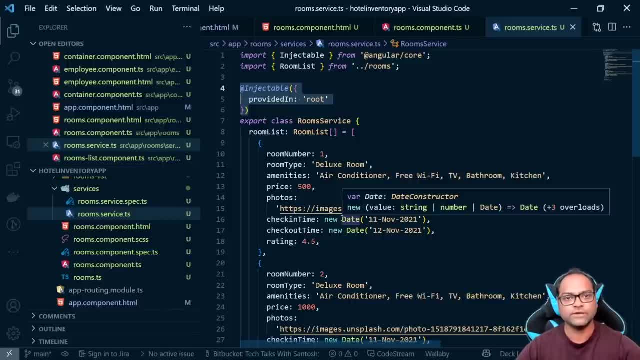 going to discuss about root right now, and any we will discuss once we go into routing, because, uh, that's, there is a solid use case which we can use. before actually we talk about this, provided in root, we have to talk, uh, something about how this particular services gets resolved. 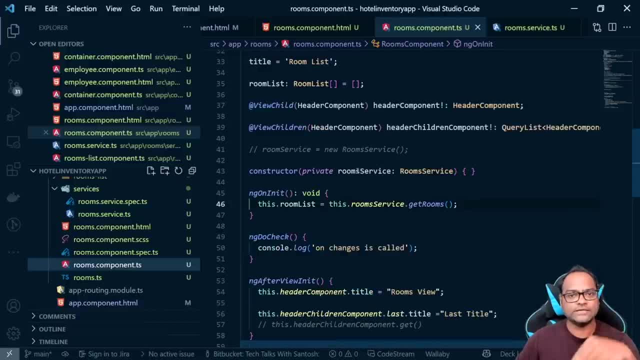 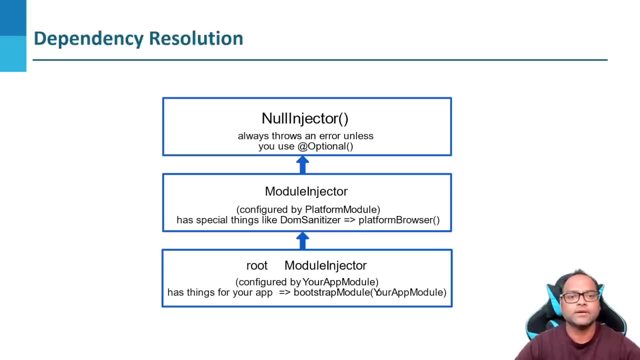 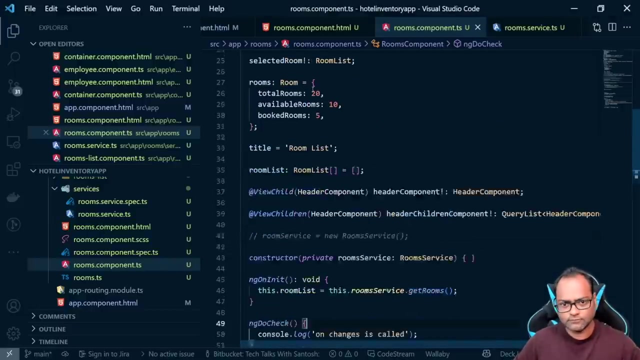 right. so we said dependency injection. so once, once we inject this particular service, angular has to actually resolve these dependencies. how we do that? how angular does that? so, to understand it, let's uh talk a little bit about this diagram, which is known as dependency resolution. here, whenever you inject a service, 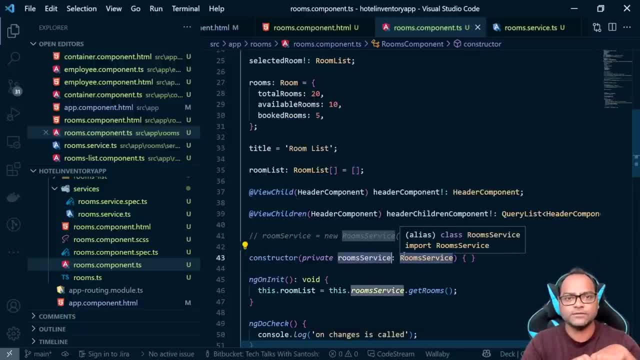 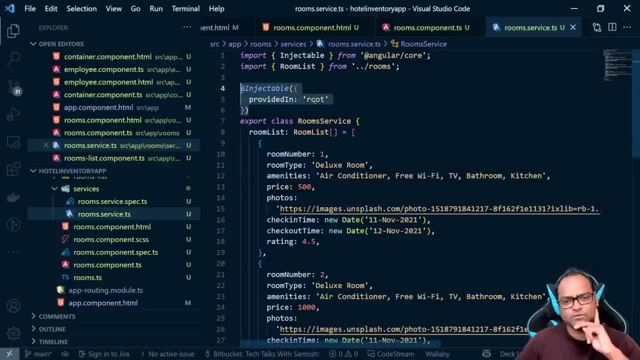 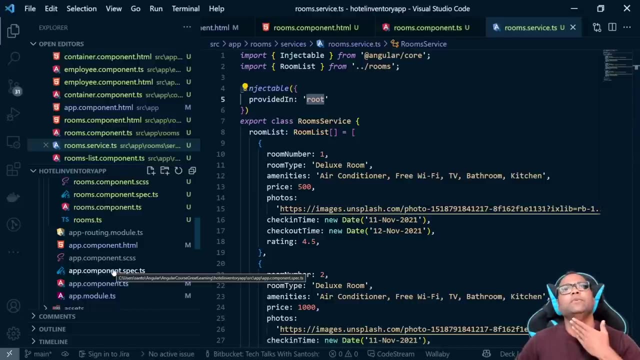 angular needs to figure out where this particular service is provided. so right now, if you see, this provided in is something which is known as root. so what? what does it denotes? in older days, i mean a before angular 6, before angular 6- what we used to do is, whenever we had, we create a wave. 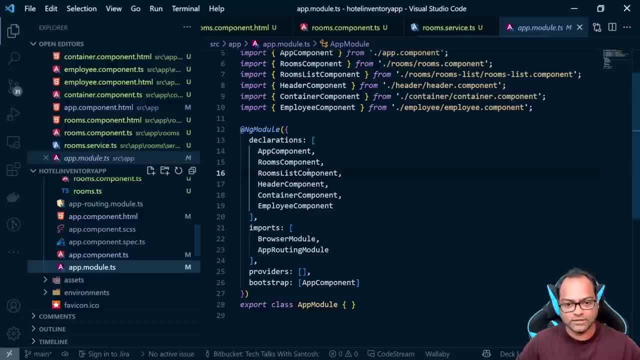 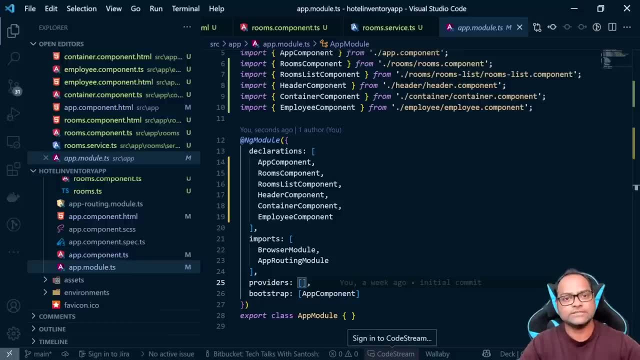 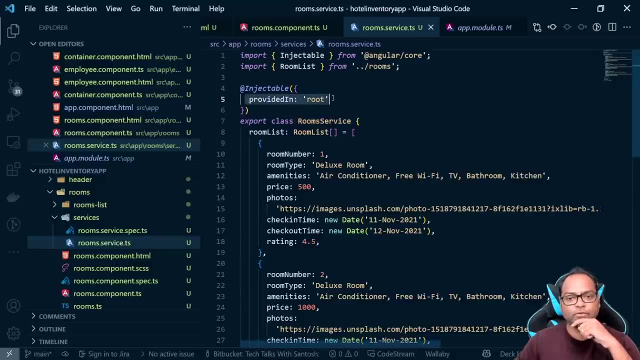 to create a service, we used to register that service here. so you can see this providers array is empty. we actually used to do it here. then, with angular 6, angular team came up with a approach where they said: when we create a service, we will say provided in route by default. so when we say 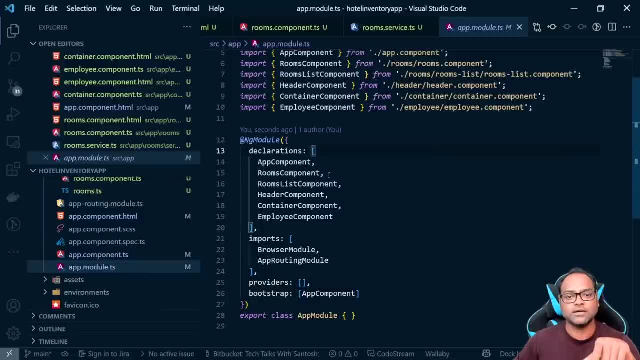 provided in route. the service is actually registered here inside this app module. you don't have to do it manually now. now why it was done, which is, of course, again very uh again, which is really important to understand so a lot of time. what we developers used to do is: 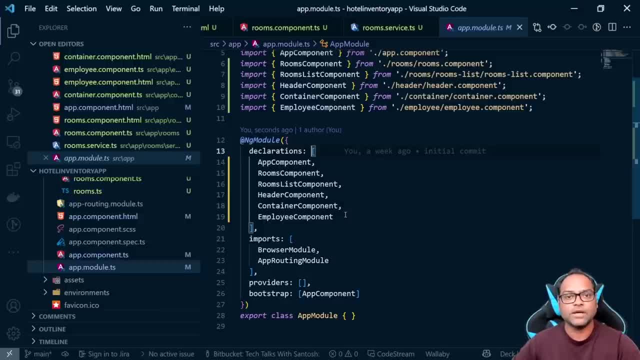 they used to inject, they used to register a service and over the time of over the time, probably after some sprint, developers used to actually stop using that particular service. for example, let's say i was doing some poc, the code made into master and now i am not using it. 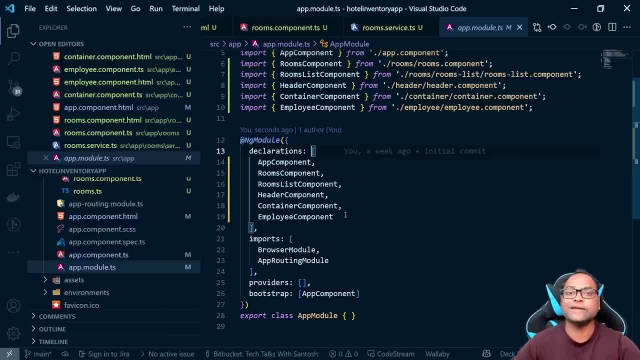 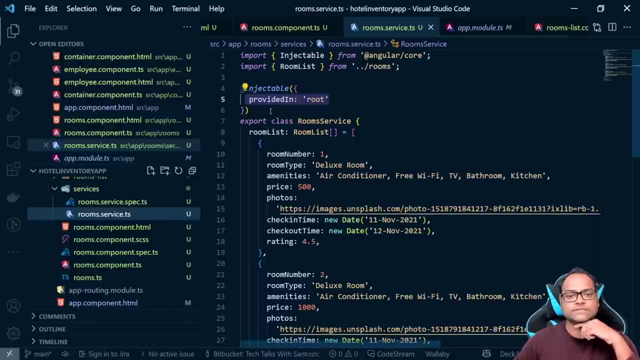 after the next release, because the poc is not needed anymore anymore. but as this is already available in providers, it is getting uh bundled as part of your code, final code. so i'm gonna set once we uh, once you create a service and say provide it in route, we will take care of registering your services here in app module. also, in case this. 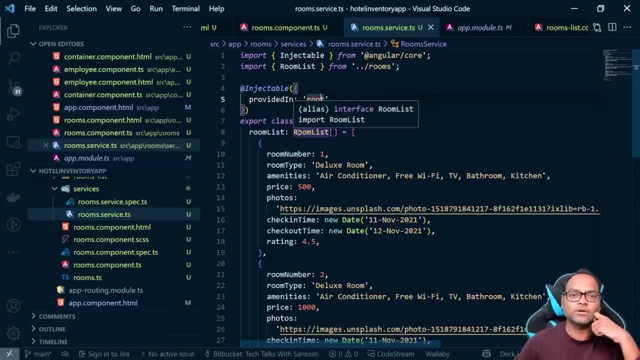 particular service is never getting used. we will also remove this from the bundle. once you create a production build win-win situation for both of us, right as framework and as well as the developers. now what else? what else provided in root does once you add a service using provided in root? 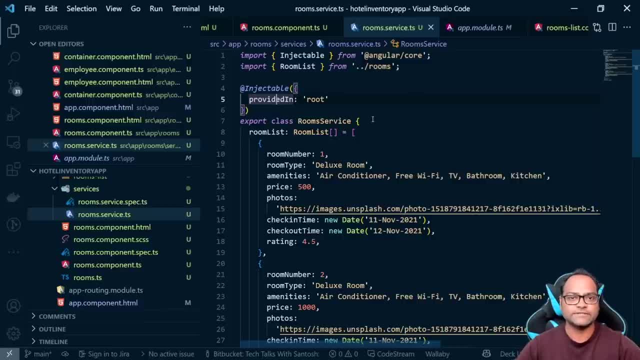 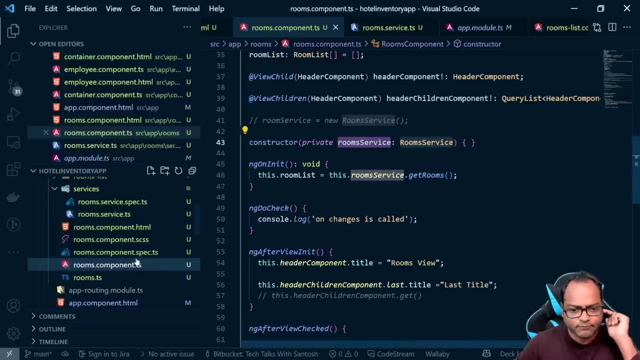 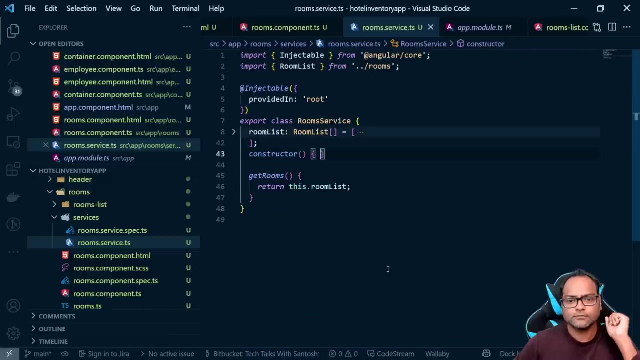 you get a single instance of this particular service available across. remember this. so what do you mean by singleton? let's try to figure that out. so what i'm going to do right now is here. let's- uh, we know constructor, right. so we, we talked about constructor multiple times. so what it is i mean, 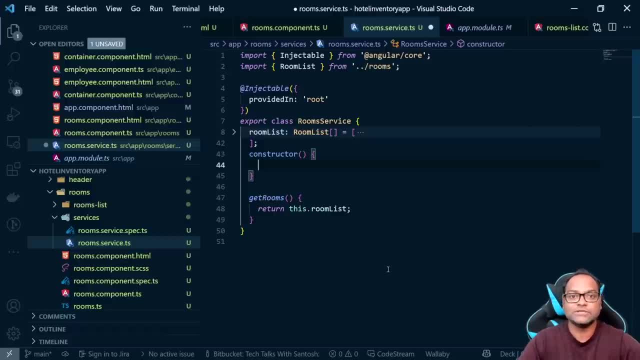 this is, uh, something which will get called whenever a new instance of your class is getting created. so here, what we'll do is we'll say consolelog and i'll say room service initialized. why i'm doing it? let's, let's go ahead and figure out. 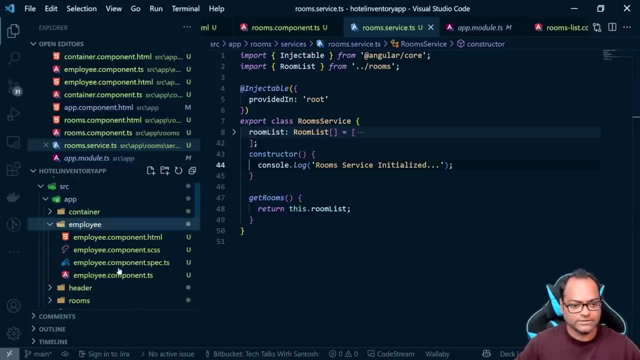 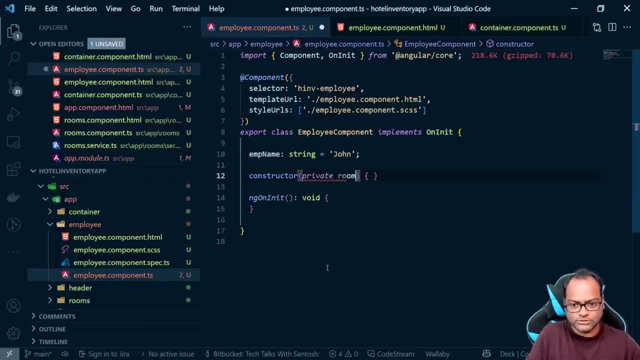 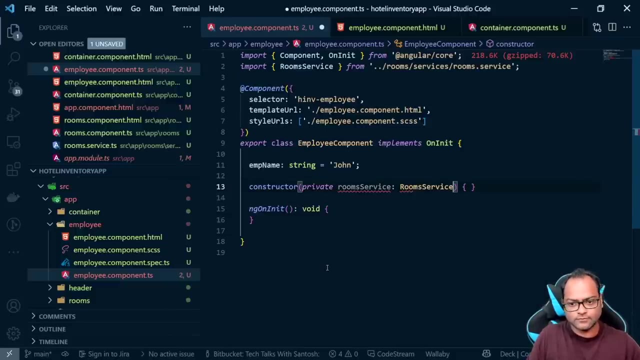 so let's say i use this particular service somewhere else, for example in employee component, and say this is private- uh, not employee- rooms service and room service. so we injected this particular service here as well. now let's go to- let's go to our view and see what is happening here so you can see rooms. 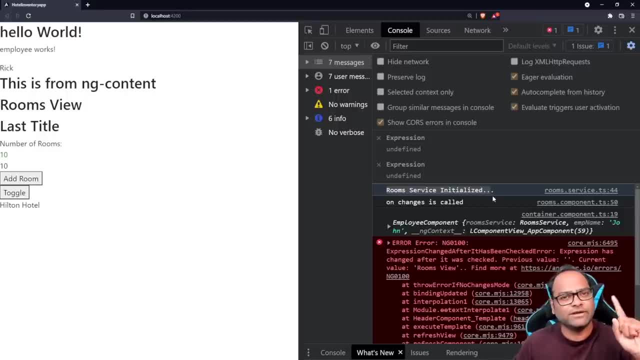 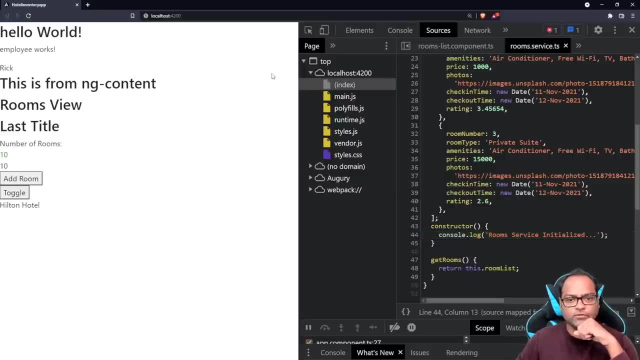 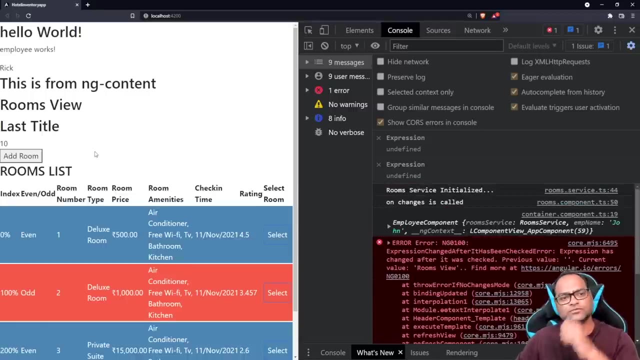 services. only room service initialized is getting called only once, not at other places, and it is from room service, this one. i mean if you even see, i mean if i click on toggle you will not see, okay, this service is not initialized again. why so? because there is only one single instance of 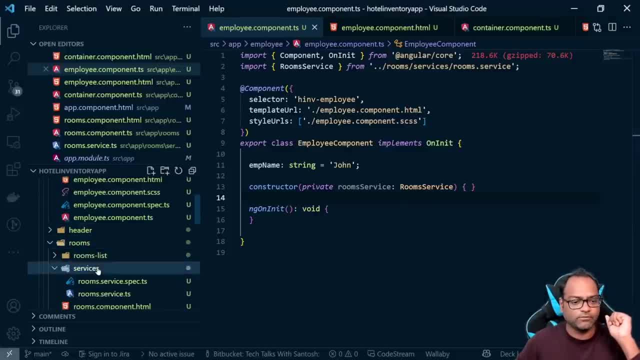 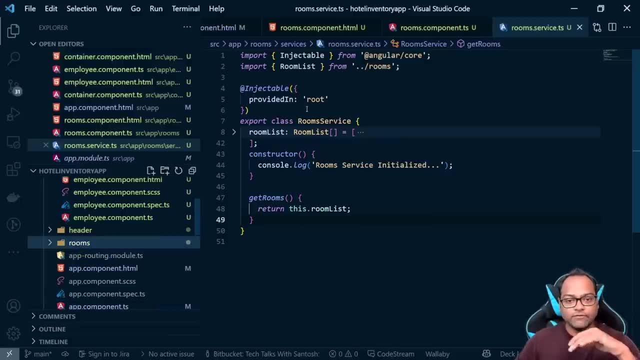 this particular class or, uh, this employee- sorry- room service which is available right now. so there is only one instance and this is the same instance of the previous one. so if i click on it now, i'm registering this particular service in my room module whenever you use provided in route. so it means i'm registering this particular service into my 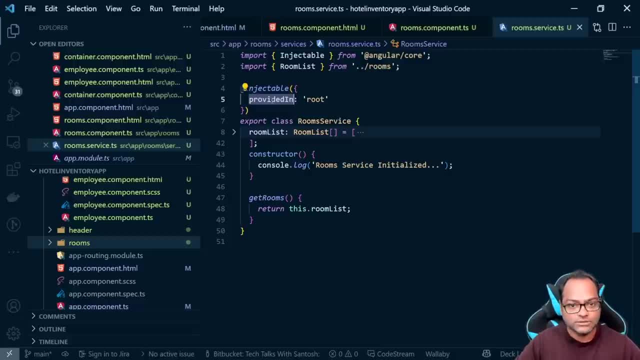 root module. if it gets used, of course it will be part of your bundle. if it doesn't get used, it will be removed. but you are also getting a single instance of your service. now let's go back and try to see what in case, i need a separate instance. 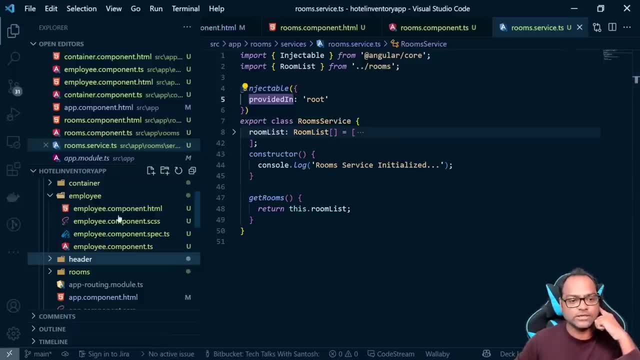 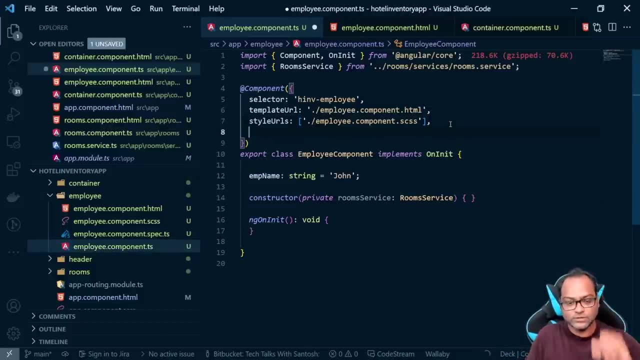 valid use case right. i mean, i don't want to use the same instance, for what I want is employees should have its own instance, So we can actually pass something known as providers, and then you can pass a service here. So I'm passing room service again here. 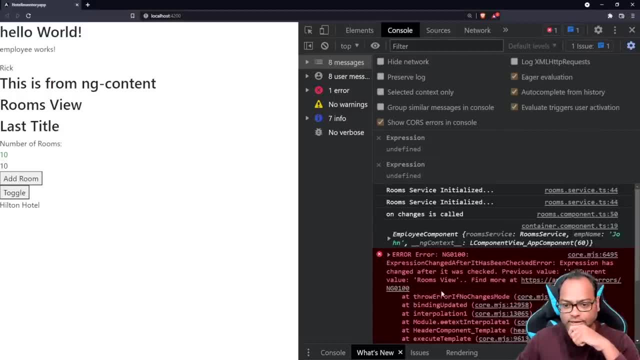 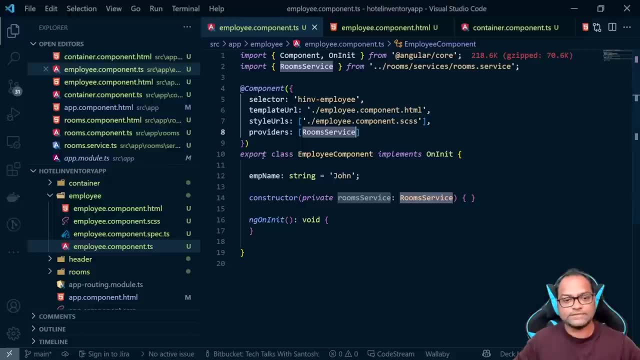 So now let's see what happens And you can see rooms service is actually initialized twice: One, of course, the global instance, Second is for employee. So who is using global instance right now- Rooms- And who is using the local instance? 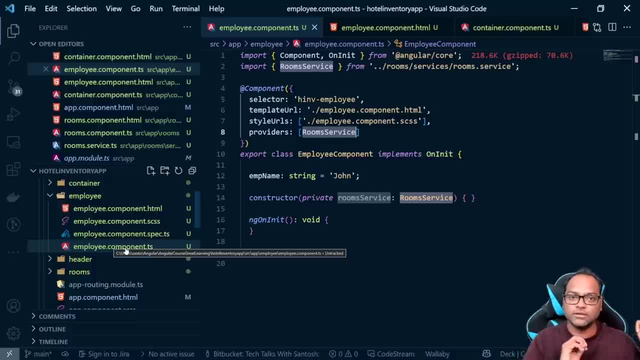 Employees. So employee has a different instance and your rooms has a different instance. So this is how you can actually create instance of your service in case you need to. Most of time, I mean single instance is more than enough, but there may be some use cases, as per your application. 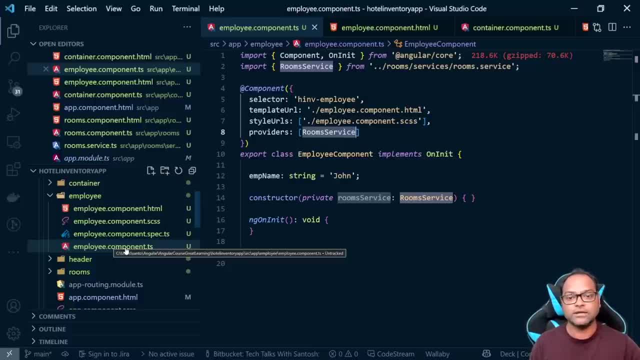 For example, a real time example which I can give is in one of the project I was part of. we wanted to actually take some JSON data and we wanted to put some controls on the UI And remember. so every screen has that JSON data. 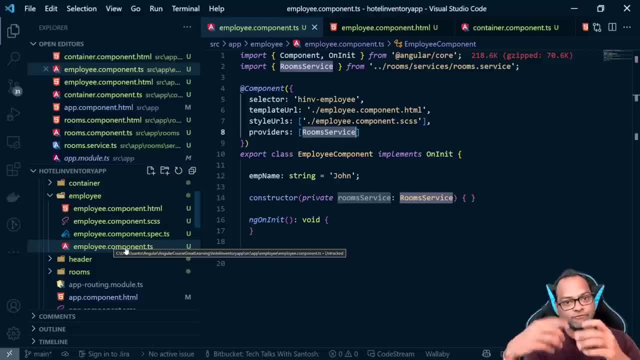 coming from the backend. So what we needed is every screen should have its own instance. So unfortunately, during testing we've actually figured it out. It didn't made it to the production, but what we did is we removed this provider's property. 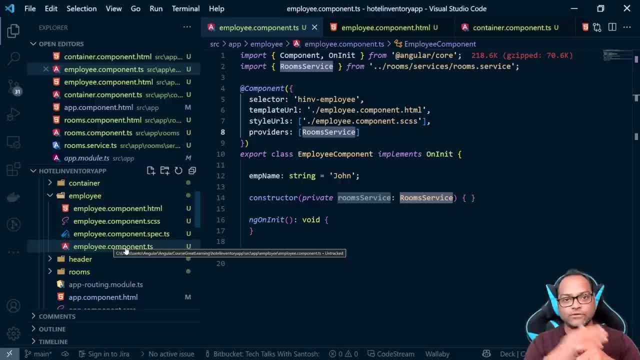 while migrating our code, because our code base was on Angular 5 and we wanted to migrate to Angular 7,, I think, where this provided in concept came in. So we ended up removing everything and then just adding provided in. So what happened is now: 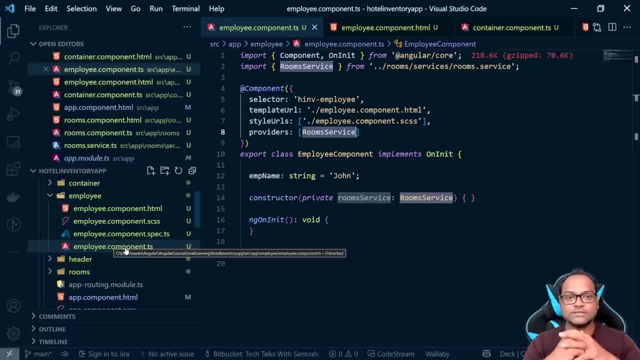 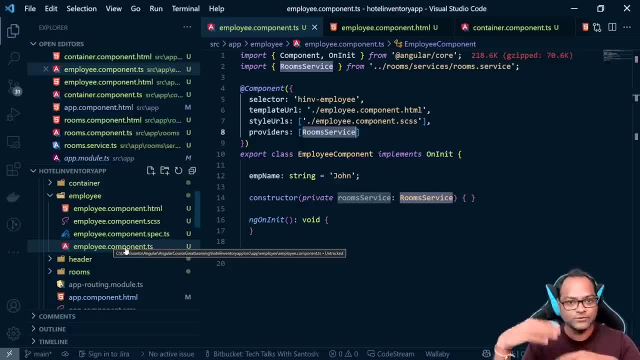 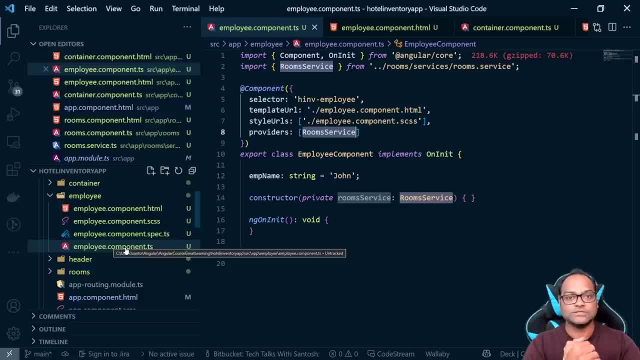 because it was a single instance. So make sure that you are sure whether you want to create a single instance or not. So, in case you don't want to create a single instance, go ahead and register your service inside that component and you're safe. 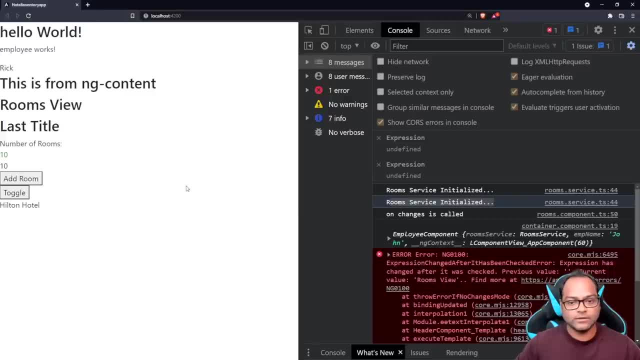 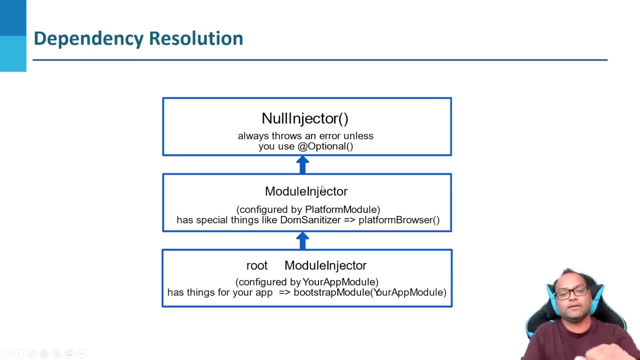 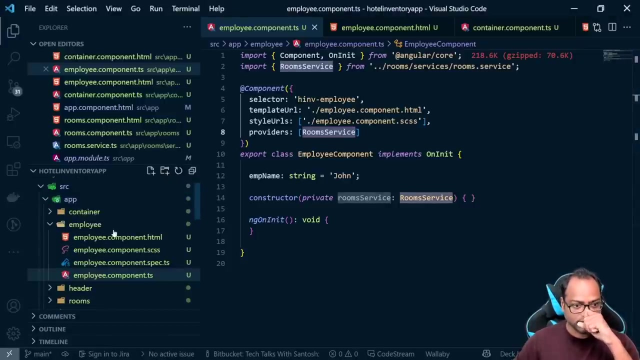 So now we know about singleton instance and how you can make non-singleton instance. Now one more thing which is again important to understand during dependency injection, So how your services are getting resolved. So here let's talk a little bit about it. 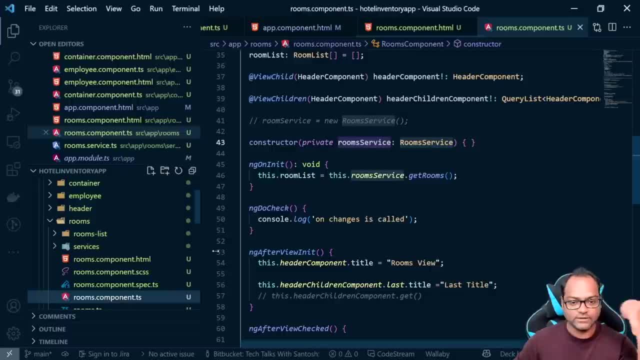 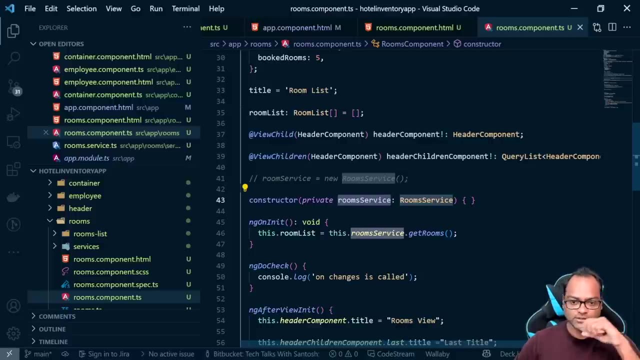 So whenever a component or a service, it checks that, OK, there is something which is injected here, The service resolution starts from this particular component. So it identified: OK, now this room service is actually injected here. First, the component will check with itself. 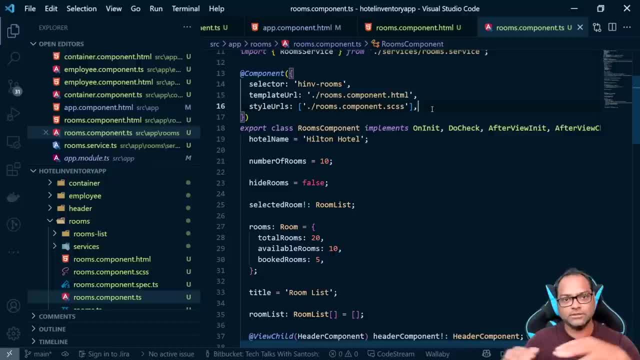 Do I have an provider's array available here? If it is available, the entire dependency resolution tree stops. If it doesn't identify that, OK, this particular service is not available here. in case I have a new: OK, this particular service is not available here. in case I have a new. 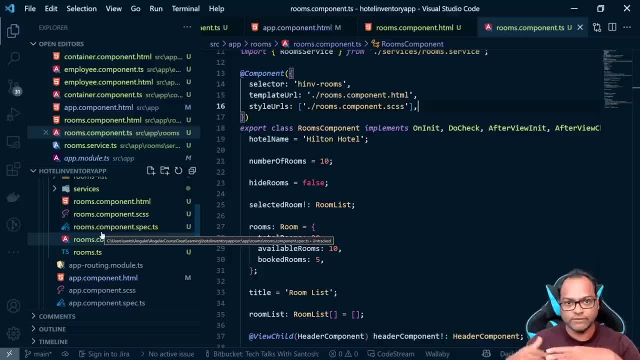 OK, this particular service is not available here. in case I have a new module. Remember, I can have a number of models. We have not just done it as of now. We'll be doing that while we move into routing. So let's say, if in, for example, rooms has its own module, 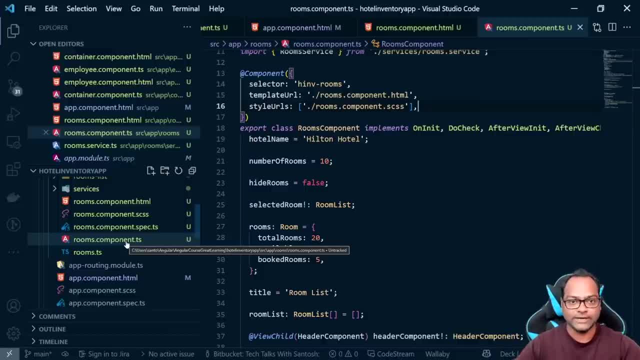 it will go to the parent, So it will be module. in that case It will check with that module- Do you have this particular service? It says, OK, I don't have it. And then it goes to the parent of that particular module. 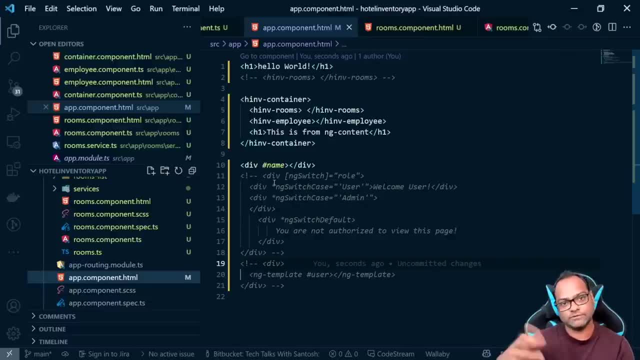 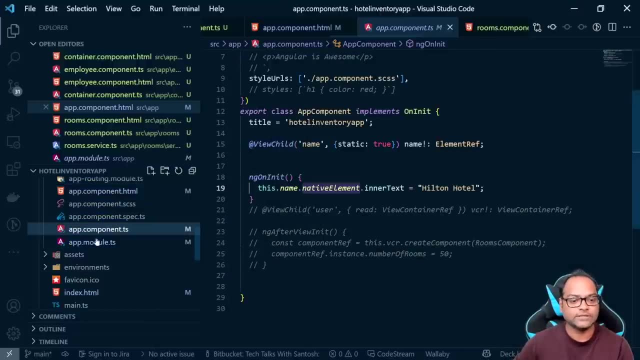 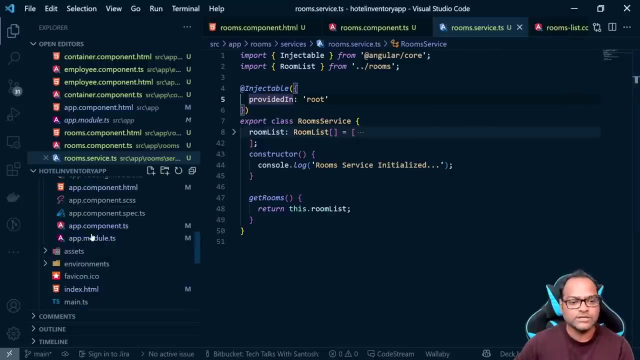 So let's say, right now we have component, app component or html, which is a root component. it checks with this particular component- do you have this particular instance? it says no and at the end it reaches to app module and, as all the services which you create are marked as provided in root, it comes here and it says, okay, i have. 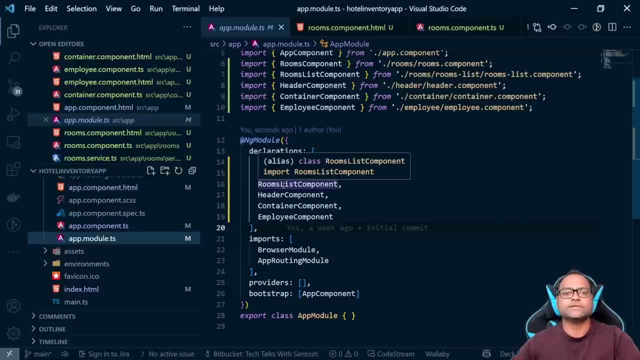 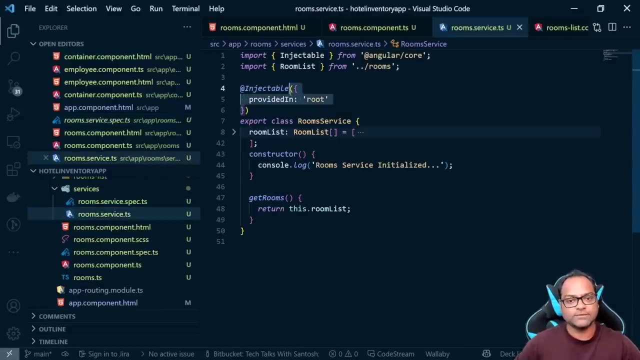 found this particular service. but in case this particular service is not registered, i mean, we miss provided in root or uh, you never had this particular property, so there is possibility that you may not have this provided in property available, in case someone migrated the code base. so what in this case? 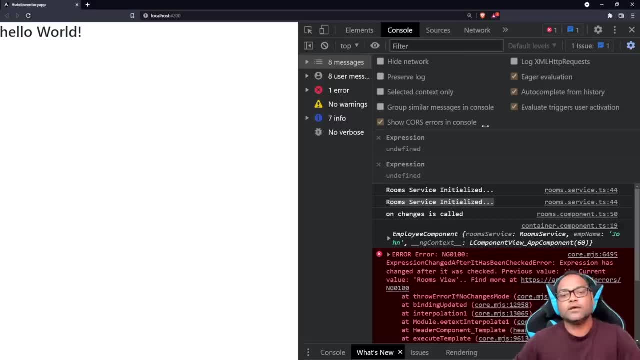 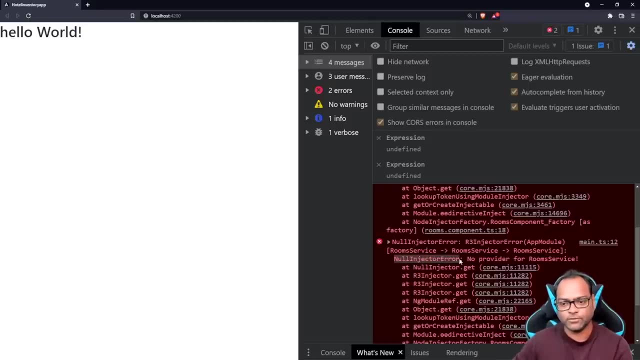 now you'll get an error. so this error is again. uh, you will find. of course, you will find a solution on stack overflow, probably on the first page. so whenever you get a error like something like this which says no provider for room service, so here it is saying. 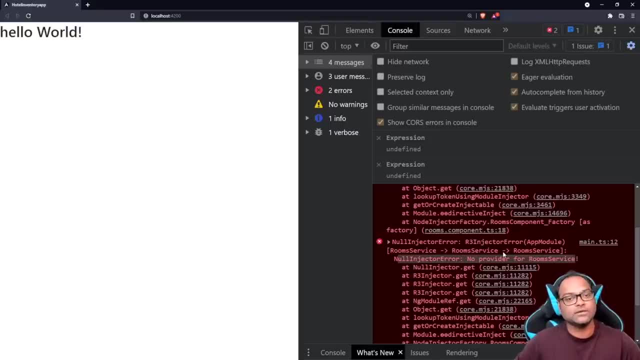 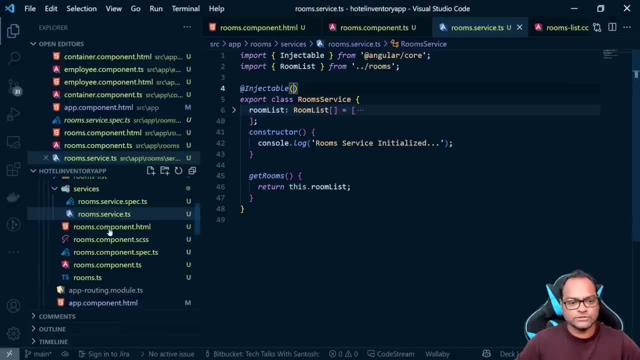 you may not have this provided in property available, in case someone migrated the code base that i am not able to figure out where this particular service is registered. remember, you may get this, of course, while working daily on your code base. it's possible. so here it is, of course, saying that, okay, this particular service was not available at app module. so what? 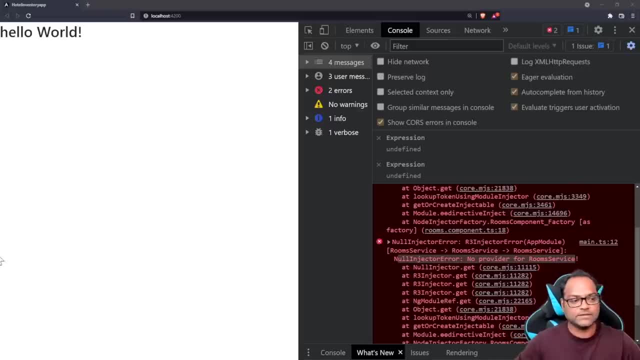 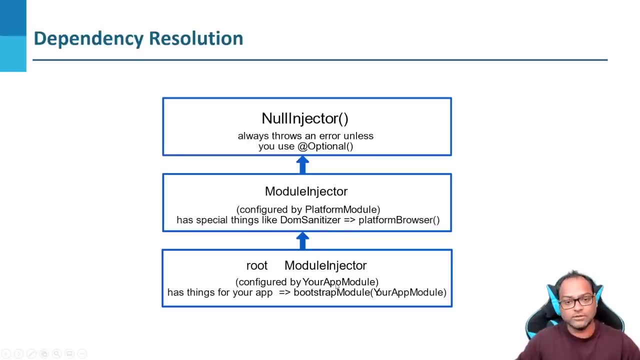 i did is i went one step above. so let's see, let's go back to the code, this diagram. so it it, uh, it actually went to this app module from our, our app module. it didn't found this particular service here, then where else it can look at lookup. so remember, above app module, we also have something called maint. 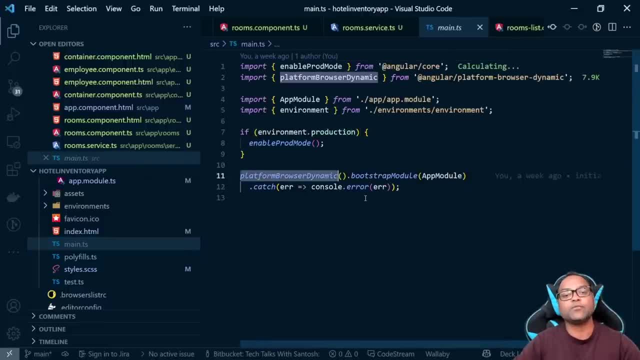 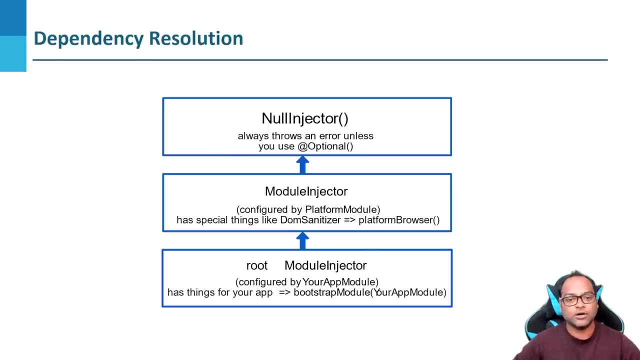 and we use something called platform browser here. so it goes to this platform browser and says: do you have this particular service by any chance? it says no, i don't have it. after this there is one more level, which is called null injector, which is actually specifically to use or check. if this 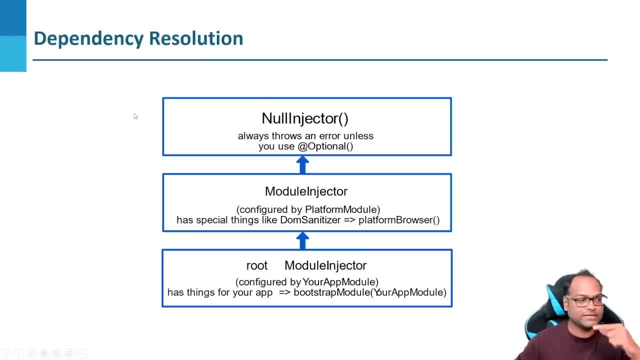 particular service is available or not. and first of all, we need to understand this service. okay, and once it reaches there, you get this particular null injector error makes sense, right, null injector and null injector error. so you get this particular error says, okay, this particular service is not. 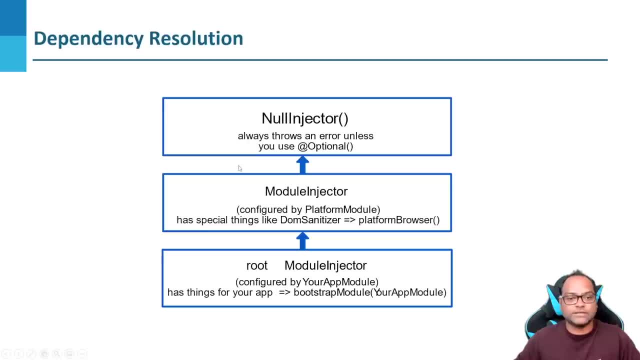 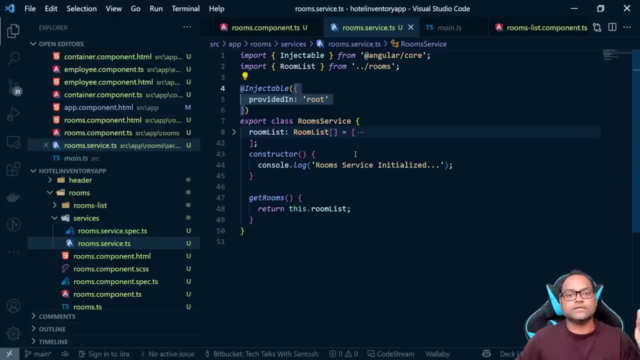 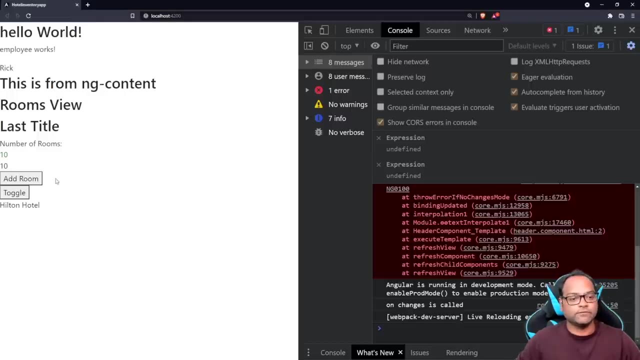 available. i'm not sure what you're trying to do, but it is not available, it is not registered, and let's go ahead and put it back, so i can go to room service and just put it back and our application will combine, will compile again and it works. so this is, uh, what this particular 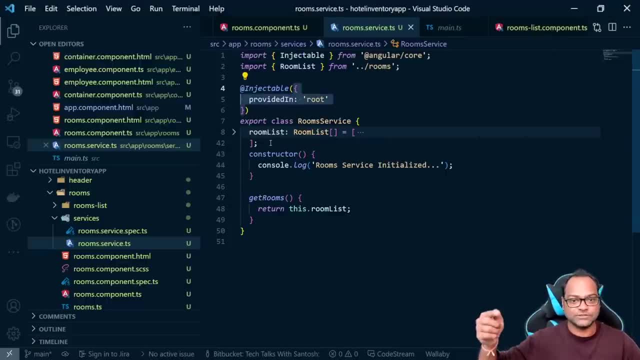 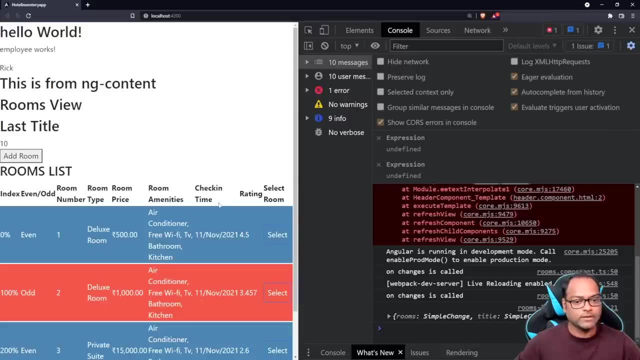 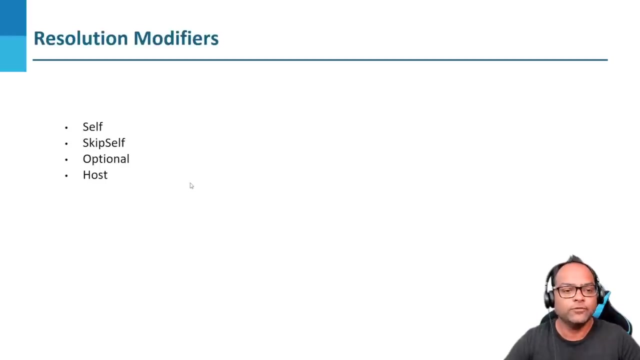 hierarchy means: so this is how your services gets resolved. so, uh, this now uh, so this is it from the dependency injection? uh, we will. we need to discuss one more thing before we end up with dependency injection and then we will move on to our gdp. so far, we have learned about dependency injection and how it is resolved, but there are 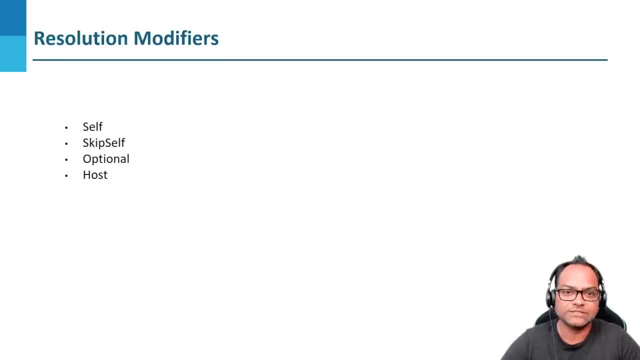 a few more important things which you should understand and which is known as resolution modifiers. so we are going to talk about four resolution modifiers, which is, which exist and which are really useful, uh, based on your scenario. so we will also discuss about the scenarios where it can be utilized. so let's start with the first resolution modifier, which is: 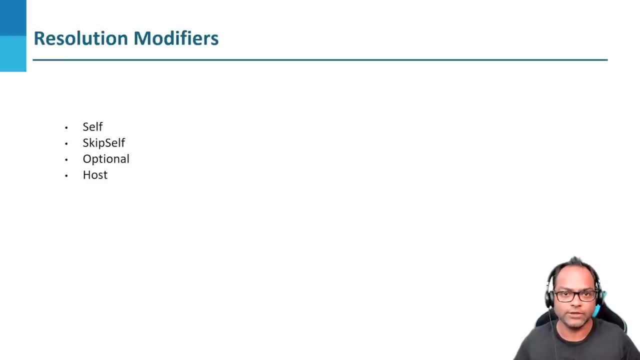 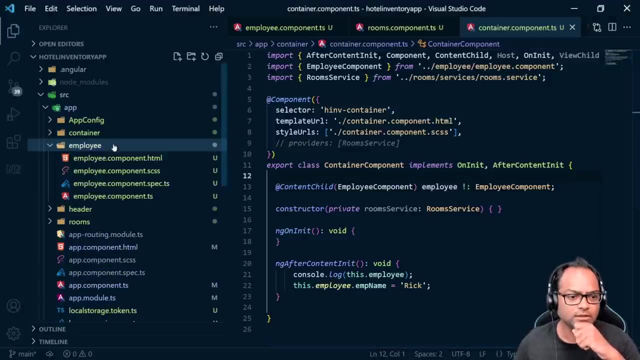 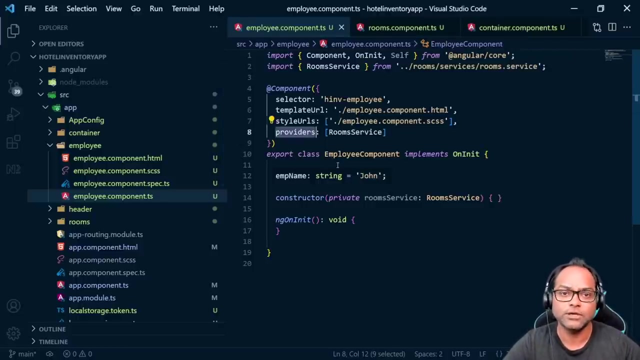 let's see a use case for, uh, this self decorator. so we are back to this code and here we will go to this employee component, uh, because i think this is the best place where the self decorator scenario uh is best suited for. so remember, we discussed about how you can actually 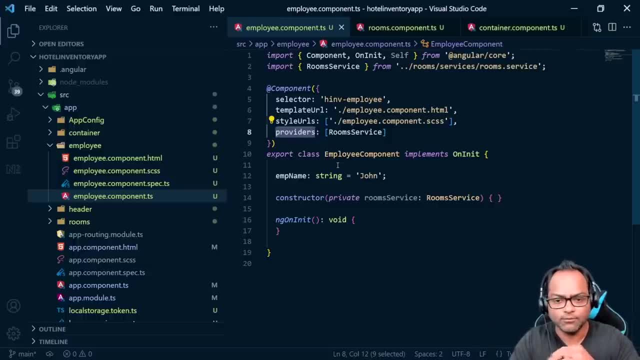 go ahead and add this provider's property on employee service because we want to have a separate instance for this particular service. and then we also discuss about the resolution. uh, how your dependency gets resolved, right, i mean, it goes to your parent and it keeps going till it finds. 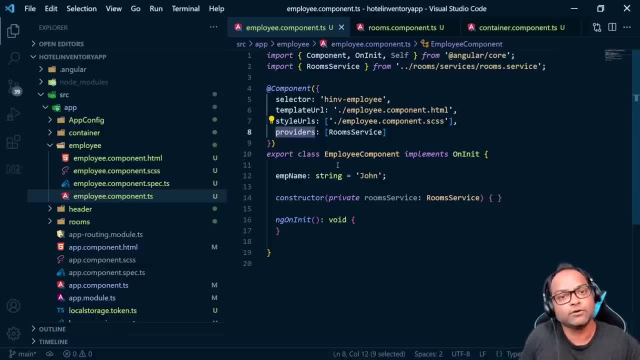 uh, the root, and if it it is not available at the root, it will go to the null injector and then we will get an error called null injector error, right. so this providers does not access, which is like, as i said widely, uh, uh, widely searched at the why it 주. I said widely, Maori search, add: only hard loop depends on the systems environment. so we have a complete service through recognized situations. this is a another of the great instance for this particular service. and then we also discuss about the resolution, how your dependency gets resolved. I mean it goes to your parent and it keeps going till it findsthe route. i mean it gives it to people brick, and also it will go to the null injectors, right too. there is many reasons to stay away from. 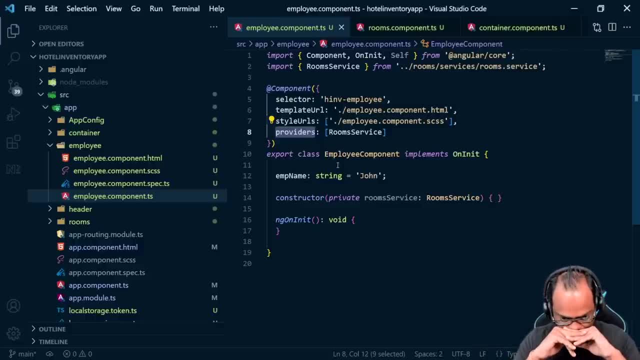 which is available on internet. but now let's go ahead and see how we can utilize the self decorator here. so in this scenario, in employee component, we are actually injecting the service at the component level, right? so we are. we are sure that this particular service should be available here. 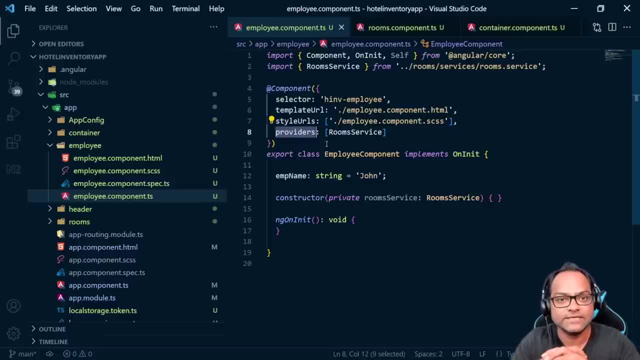 that's the use case and that's the expectation as well. so what we can do is: we can by using at the right self decorator, which should be imported from angular core. remember this. by using this, we can by using this self decorator. now we are saying that this particular service 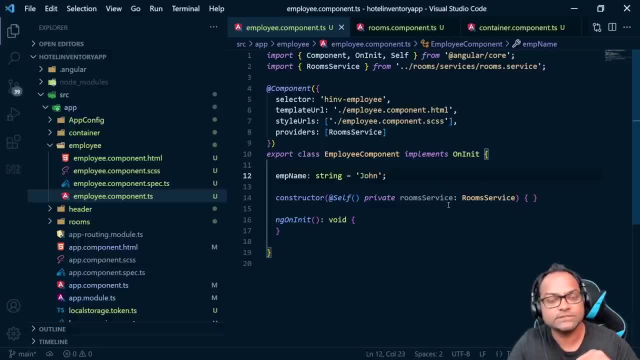 should be available at this level. if this particular service is not available here, it means we should throw an exception. now, when it can be available at this level, we can use this as an exception. now, when it can be available at this level, we can use this as an exception. color. 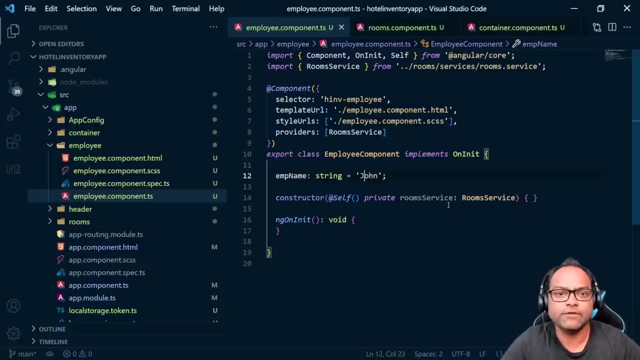 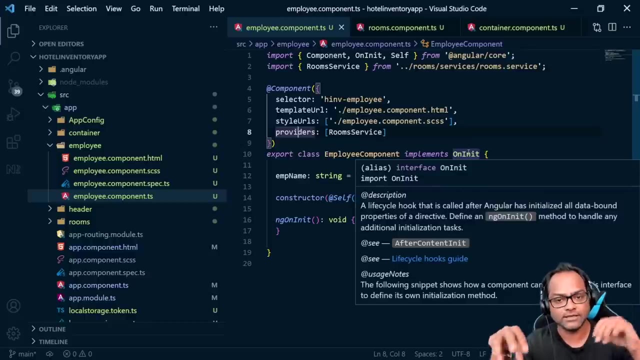 so, for instance, set up our new section and we can type in check in uh text also we can entered for if we could file in uh two Neweren and under text by entering IDS into the box and По copy right now. after we click on it, u can see that the new settings. 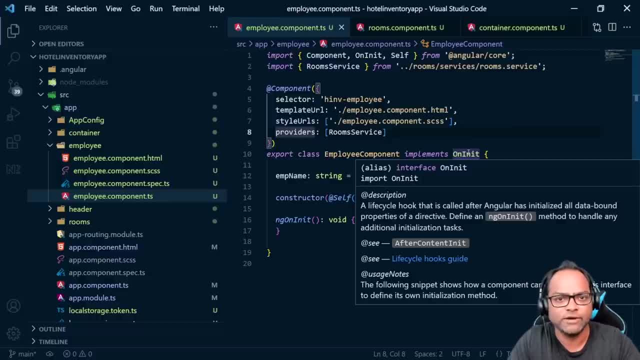 will appear on top of the file. As soon as we click on it, this empty box immediately shows up and it's going to be sent to your server. For before I Ya Iized it here, property came around Angular 6.. So what we did is, by mistake, we removed that property. 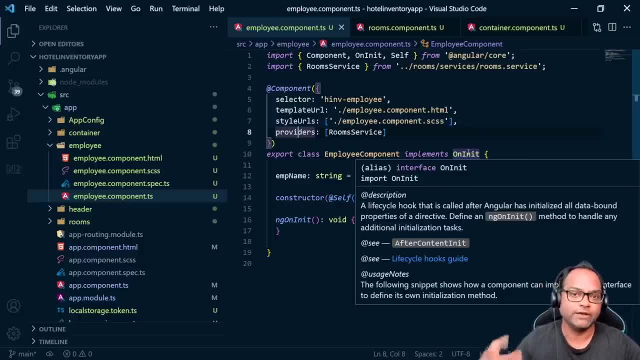 And what happened as we removed this property. whenever we used to actually revisit different forms, all the controls used to get added into the same service because it was a single service And at one point we realized that our form, one of the page or one of the form, is really slow. 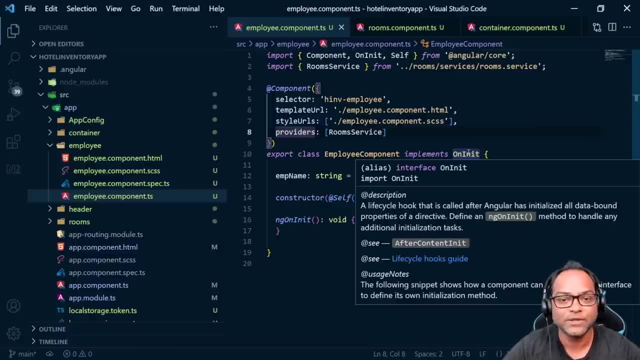 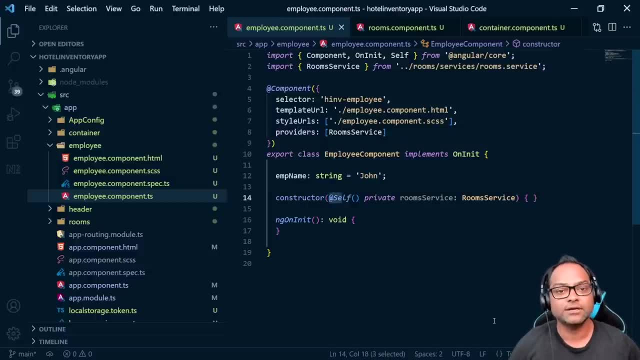 And then we realized that, okay, behind the scene it has like 300 controls. So that was the use case, But in case we might have added this self decorator. it actually serves the purpose, because it should tell us that. okay, now this particular. 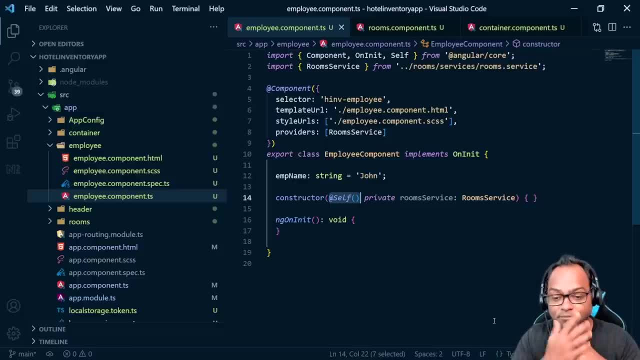 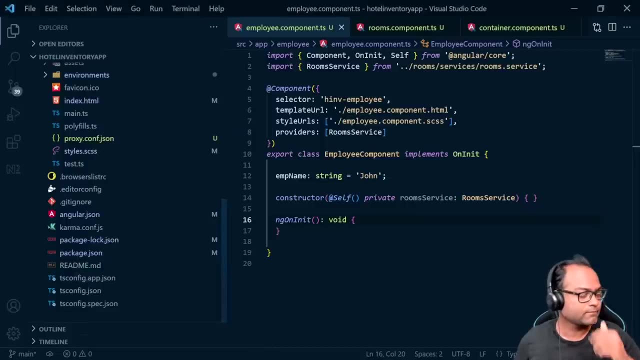 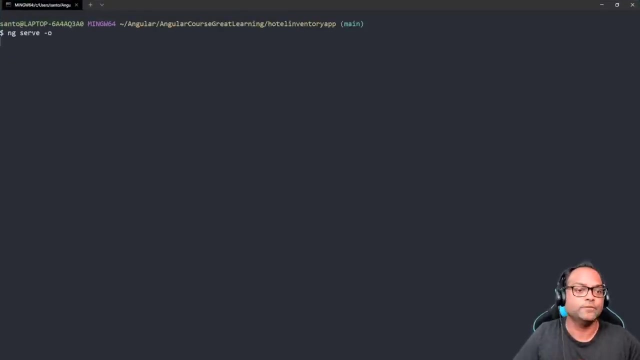 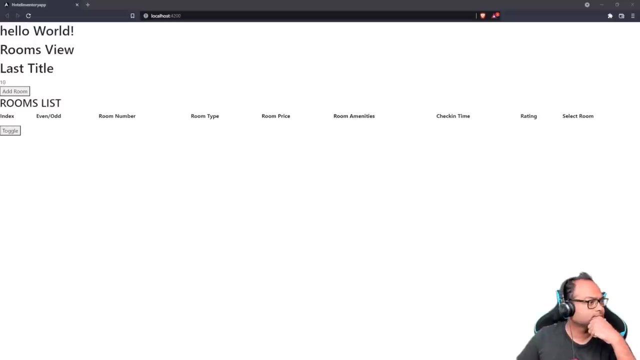 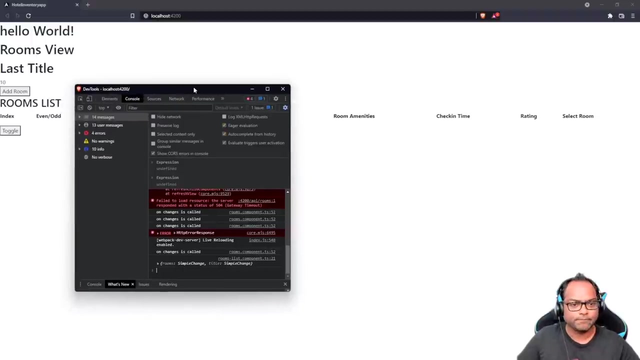 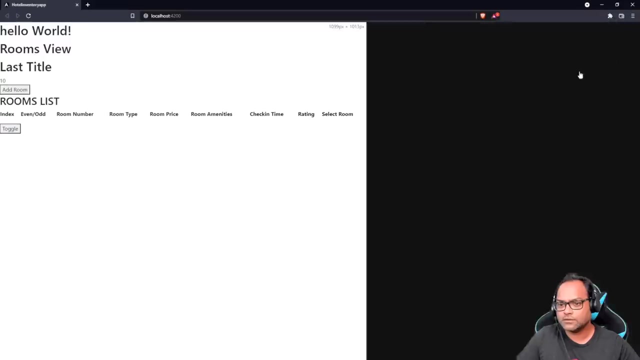 service should be available here, should be registered here. If I use this self decorator, let's run this application first. So I'm going to run this application, So the application is here and let's click And let's keep it side by side because we want to see the error. 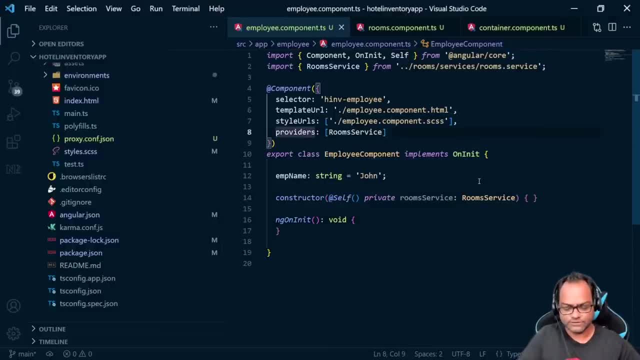 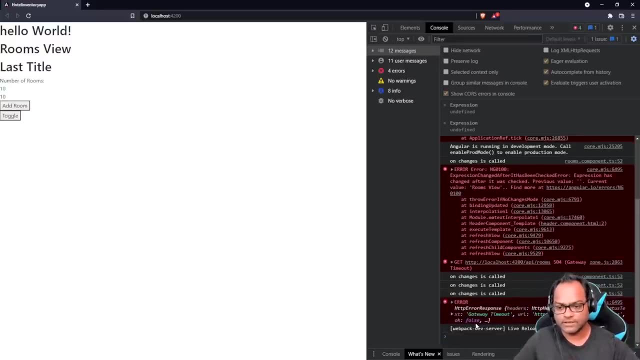 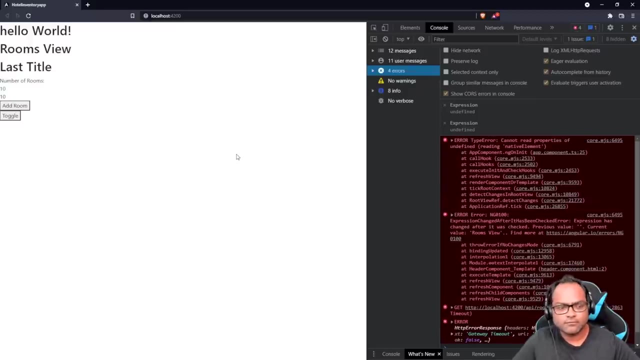 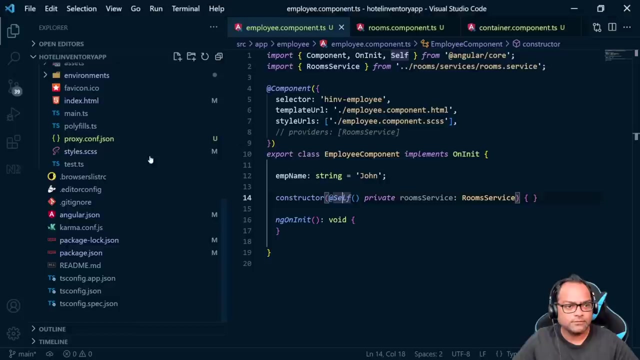 So let's say, if I add the self decorator and I remove, this provides property. So now what we'll have Is we will start getting the same error which we have received earlier, which says: let's come back here. Okay, Looks like this employee component is not available. 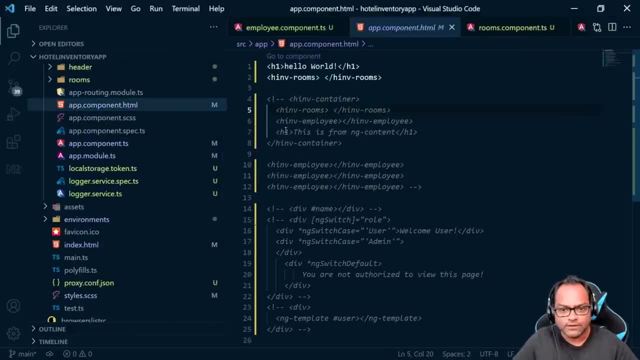 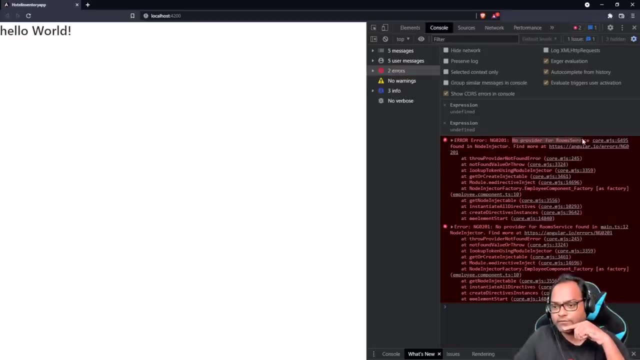 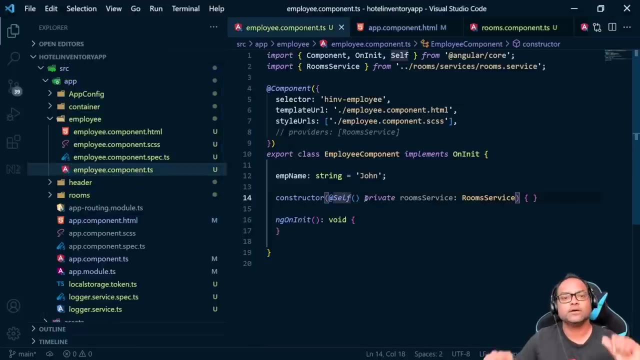 That's why I just add this employee component somewhere. Let's add it here And now we have This: no provider for room service, right? So we started getting this error Now actually here, as we added self decorator now during uh or file resolving this particular. 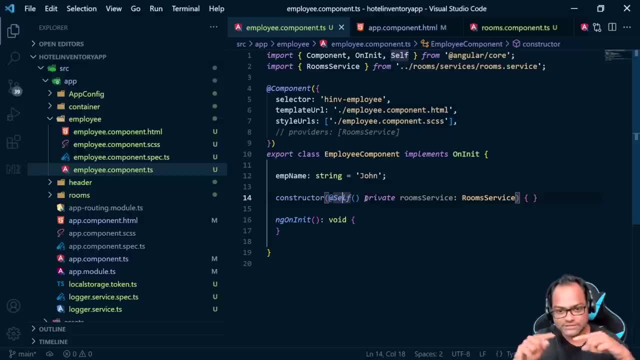 instance, angular will not go up. It will just try to see if it is available here. If it is not available here, it directly goes to the nail injector and it traces an error that this particular service is not available. So, pretty useful, pretty useful in case you are aware that, okay, your service will be, you know. 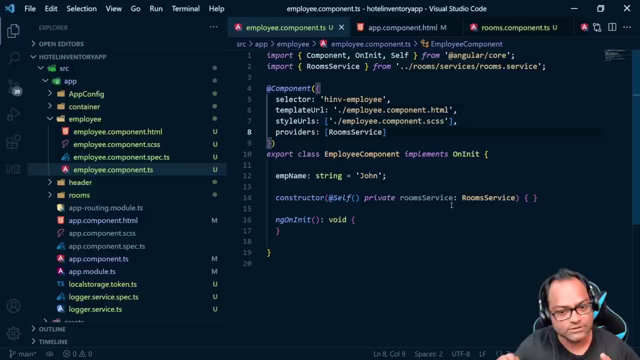 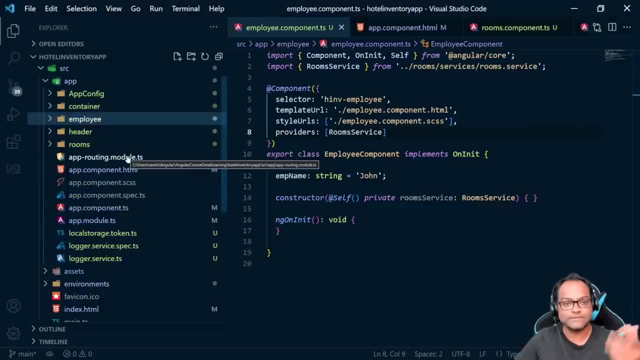 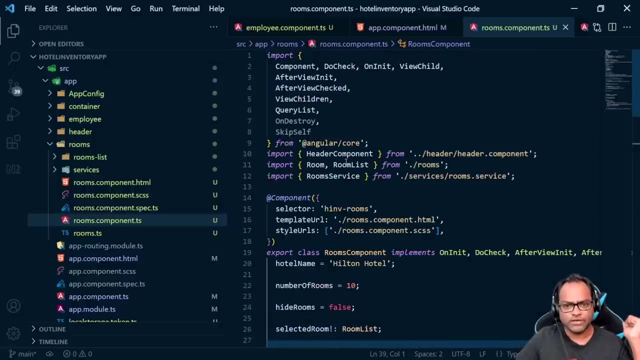 your service will only be registered at this particular level. Go ahead and use it. Now let's move on to the next decorator which we have, which was skip self. for that, We will take an example of this rooms component service, because if you see, uh, we are not. 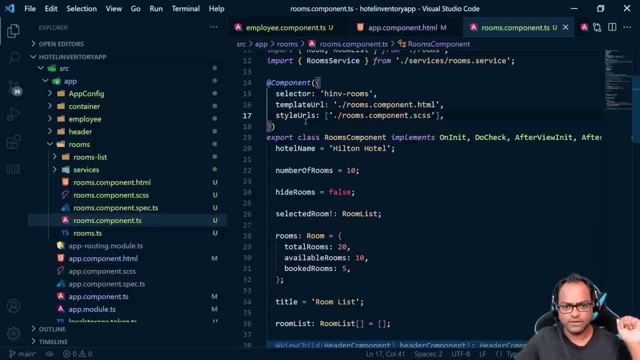 registering the service here. right, We are not saying, okay, this service should be available at the component level. We are expecting this service to be available somewhere. I mean, maybe his parent, uh, parent of room component, maybe app component or app module. 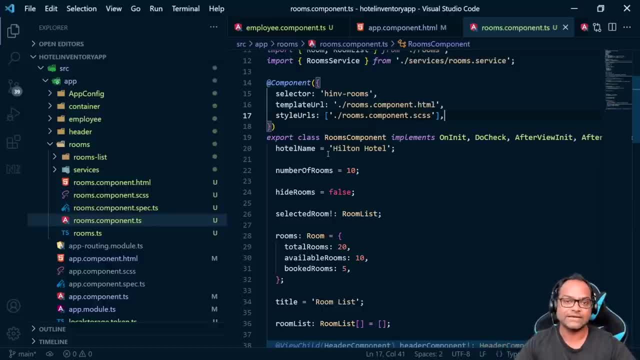 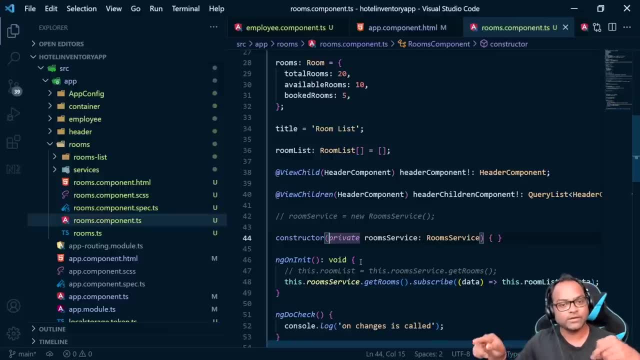 So we are aware that, okay, this, this service, will never exist at this level. So what we can do is we can ask the angular to skip the check for this particular component by using skip self. That's the name, right, So name itself suggests skip self, skip myself from the entire dependency resolution tree. 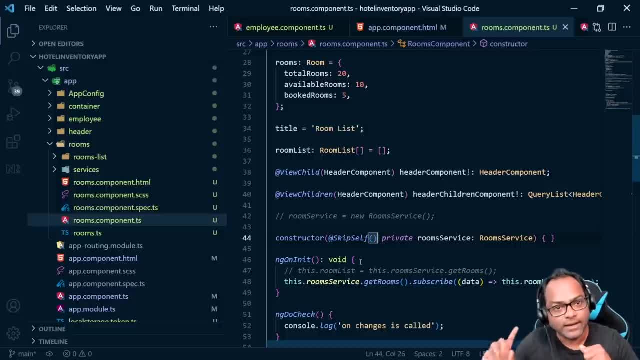 which you are going to execute. Skip myself again. Give you an idea? Do we, should? we use this? The answer is: maybe because angular internally, because angular internally uses something known as blue filter to figure out where the service or the instance is available. 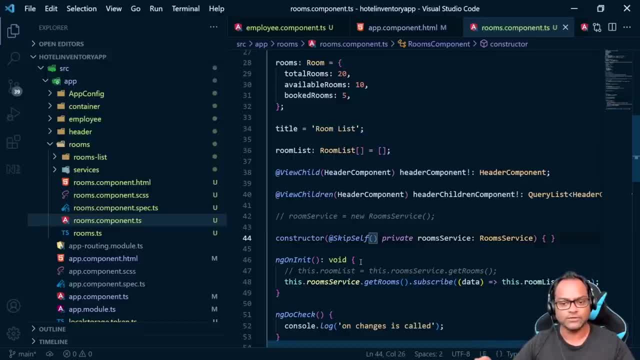 And it is pretty fast already. You don't have to do a good end, You skip self, but it is a useful uh. fifth, another attribute or another resolution modifier called optional. So let's go ahead and see Uh next. 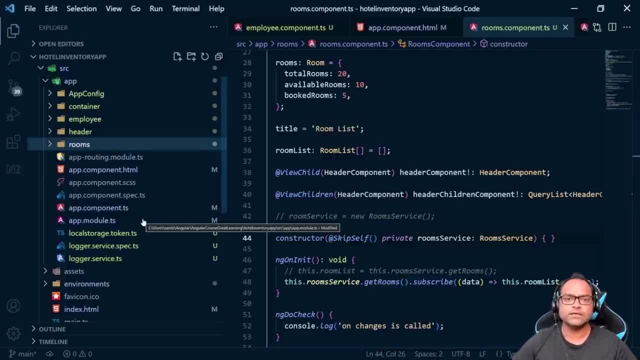 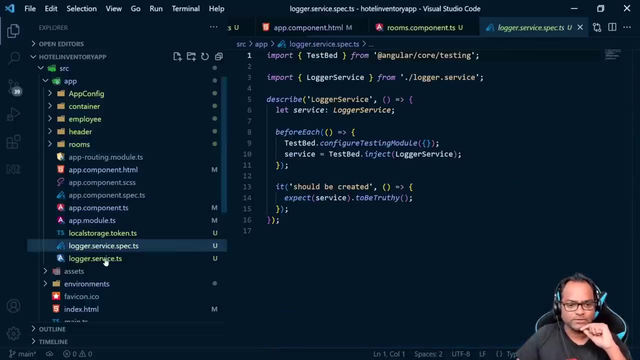 Now the next attribute which is available. we will see optional first, and then we will go to the host To understand the optional one. what I have done is I have created a service called Logger, So this is Logger service and it. 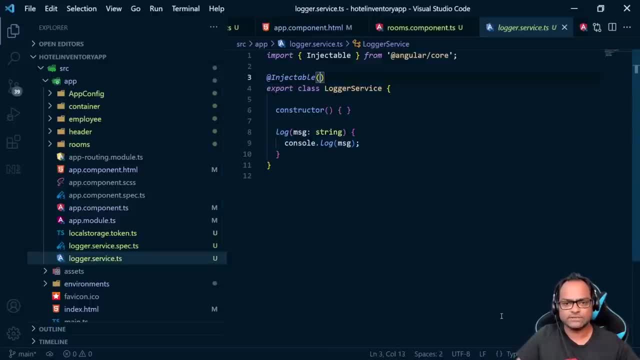 contains a method called log, And you can see what I have is just add this- provided in property here, because I have moved it right now. So I have created this new service And what I'm going to do is I'm going to use this Logger service, but what we need 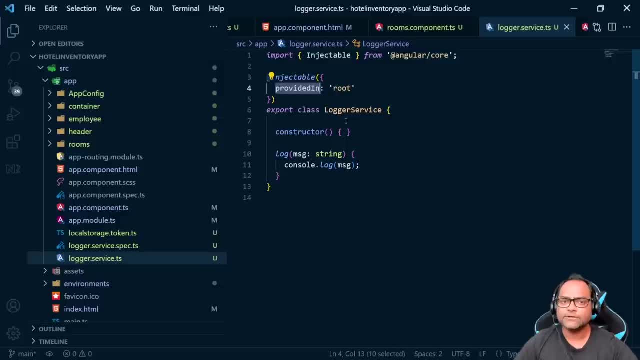 is: we want to use this Logger service only during dev environment, During production. actually, we don't want to use this Logger service But, as we have seen, if we try to remove this provided in property, we will get an exception, because we are seeing if this particular service is not. 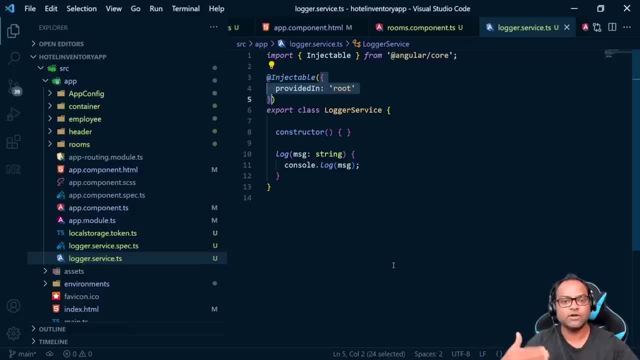 registered anywhere. go ahead and raise an error. Even though we use skip self or we use self, we are going to get this error. So this is what we can achieve using optional decorator. So let's go to app componentts. We will actually inject this particular service here. 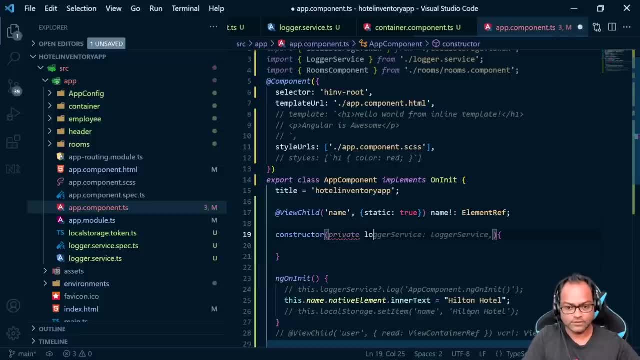 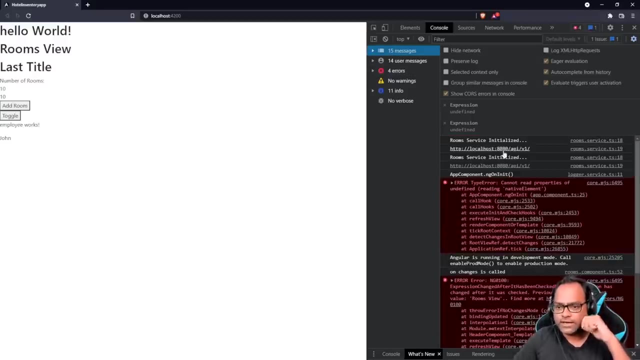 So let's say private logger service, which is type of Logger service, And let's uncomment this. So I'm going to call this log method and let's see, And we have this app component. So this is something which is logged at this line. 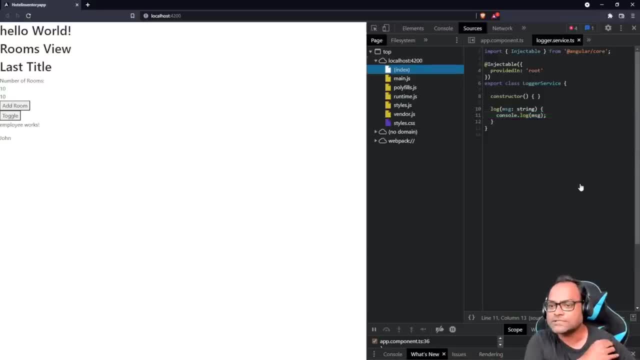 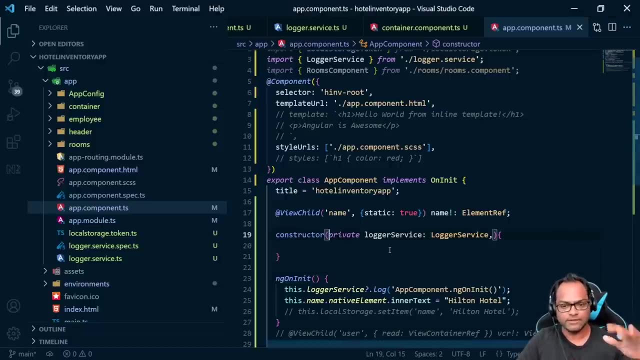 Angular, you can see LoggerServicets, But during production, let's say we don't want to inject this service. I mean, there are multiple ways. We will not talk about it right now, But in case, just to recreate the scenario, 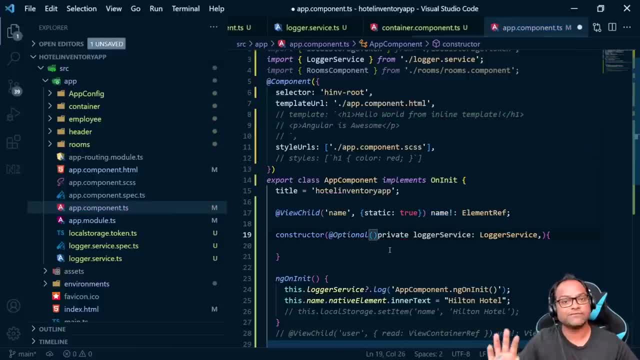 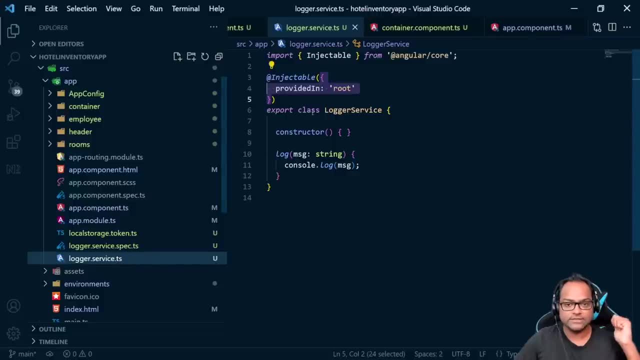 where this particular service is not registered. what we can do is- let me just add optional later on- but we can actually go ahead and recreate this scenario where this service is not registered. So we can do this- Let's say this service is not registered, by removing this. 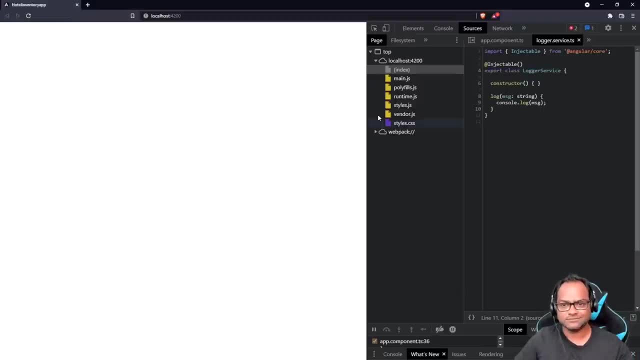 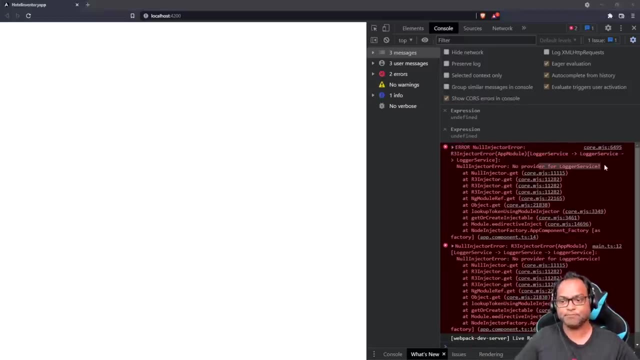 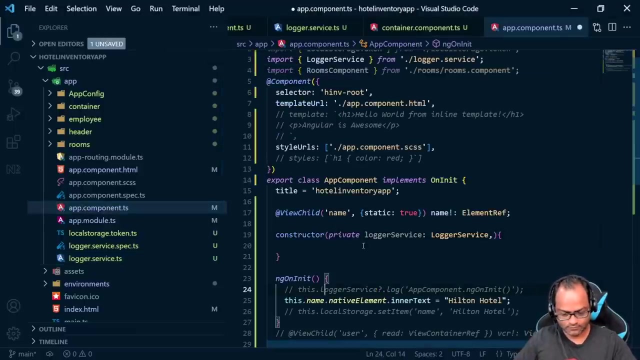 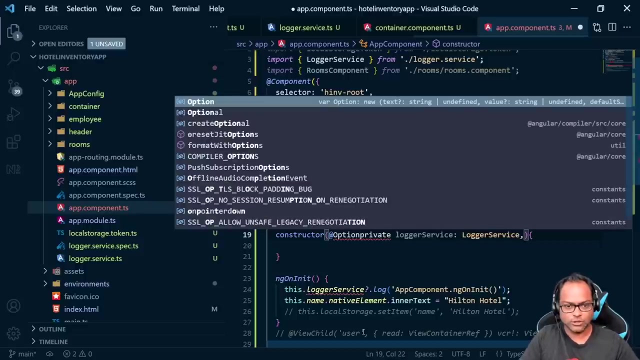 provided in root property. Now we will start getting an exception saying this service is not available And no provider for logger service. this was expected, So what we can do is we can mark this service as optional, So let's go ahead and use optional decorator. 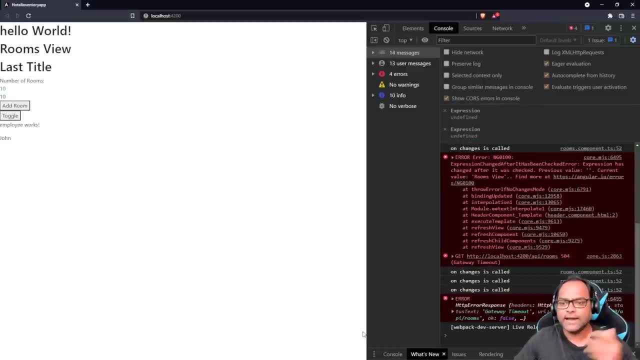 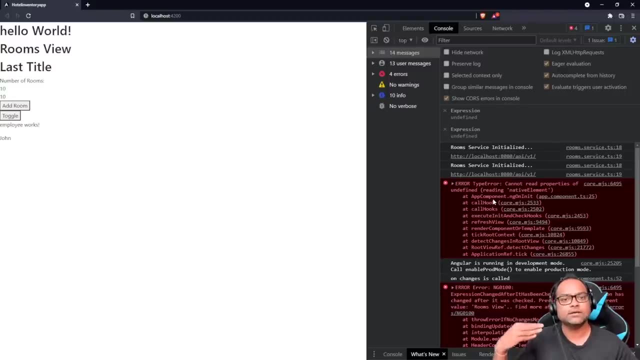 Not option, Optional decorator. And now let's go ahead and see And the error is gone. So we don't have that no provider for logger service anymore, because this is optional. So in case Angular figures out, there is an instance which is available, it's OK. 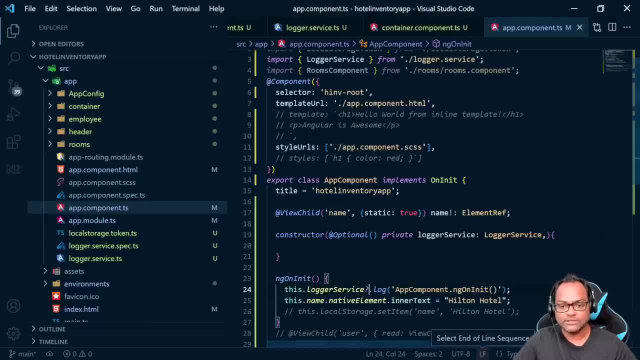 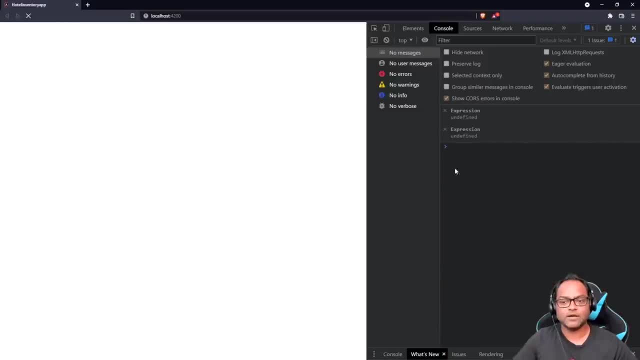 If it doesn't just go ahead and execute it. I'm using this ternary operator here because, in case this particular service is not available, we will get an error. So let's see. So if I try to execute the log method there. 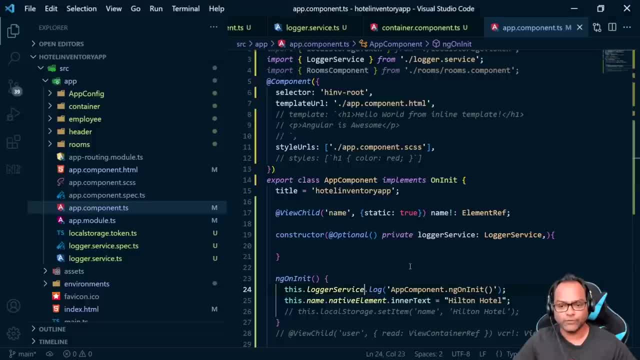 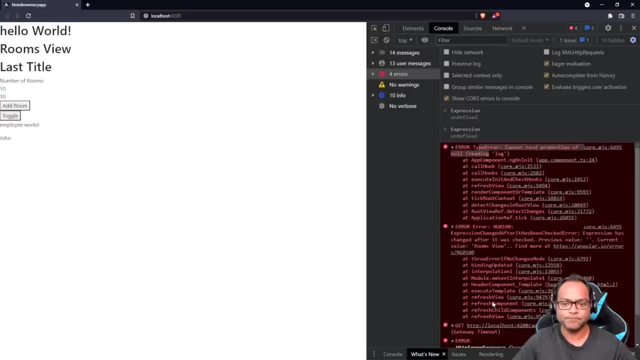 you can see, cannot read properties of that. So to avoid this, I'm using this ternary operator, which will only execute in case logger service exists. Otherwise, it will just skip that. So this is optional. Now, what we will do is we will go ahead. 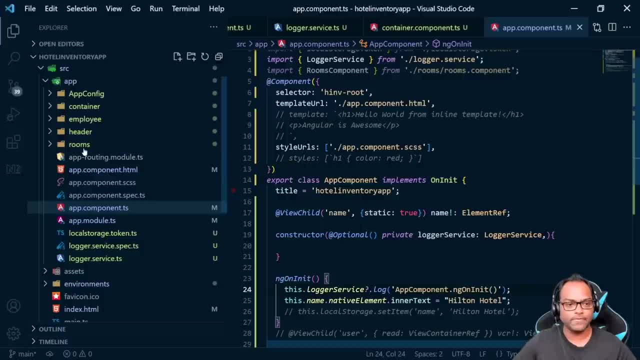 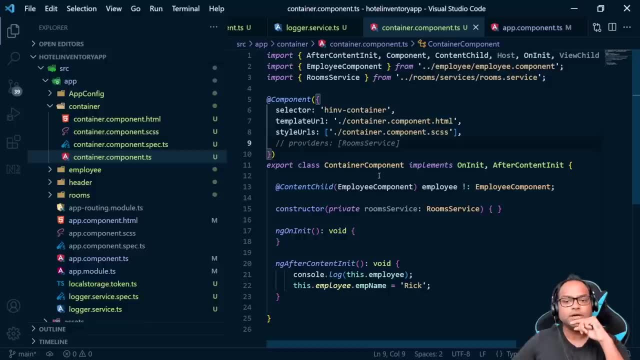 and see the last decorator which is available, called host, And for that what we are going to do is we are going to take this container example. So what we have here is we have injected this room service here In my container. 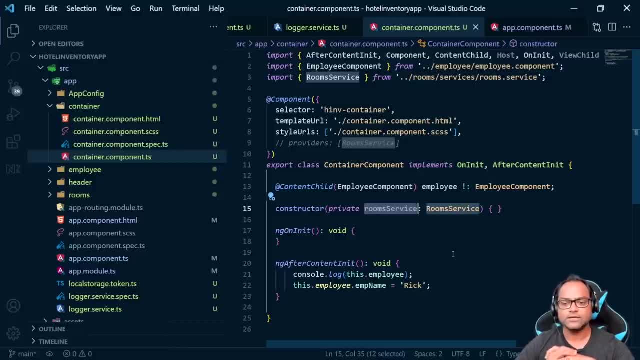 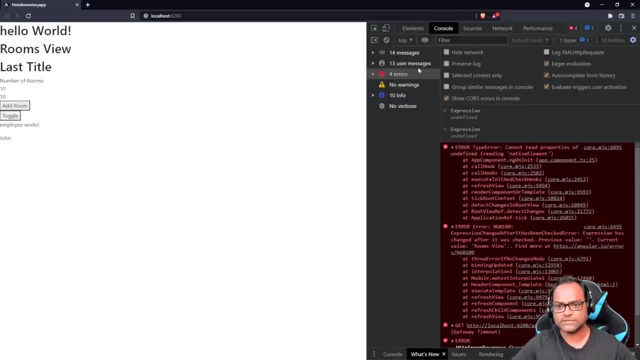 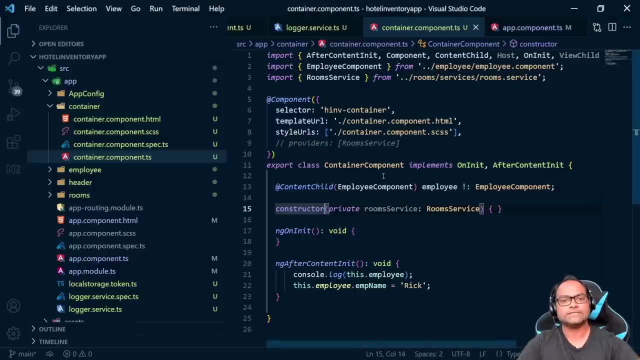 Now how host is useful. let's talk about that. So here, how many instances of room service which we have, Let's go ahead and see that. So we have one and two instances right now, In case I want to have a separate instance. 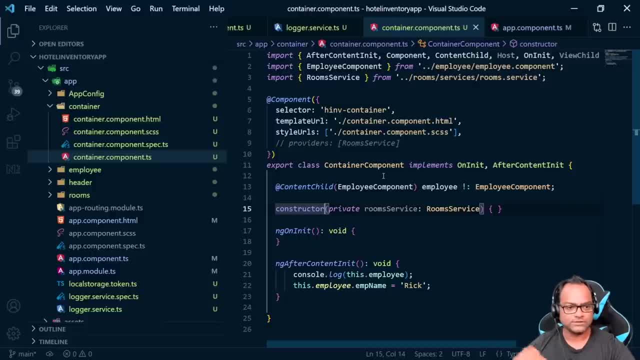 for all the components which are part of container, like this container component. In that case, what I can do is I can just register this particular service here first, And then I can add the host decorator here, Now all the component which is actually. 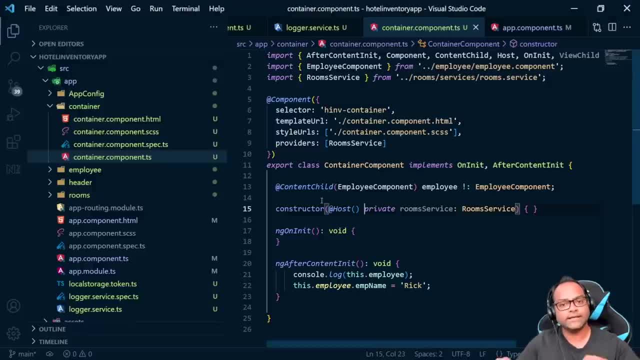 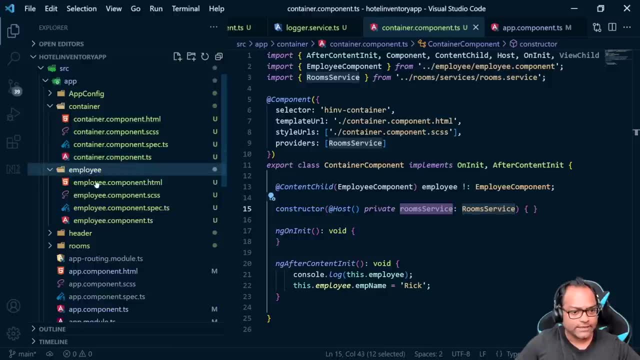 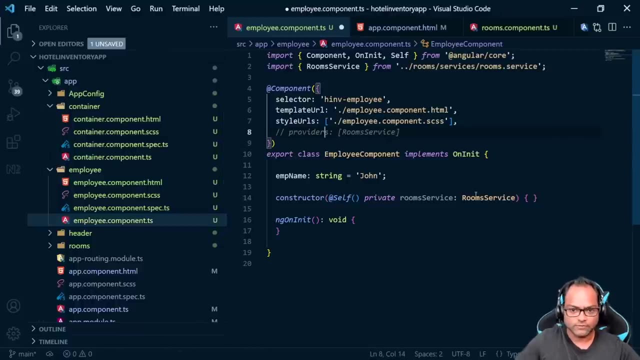 loaded inside this particular container will start using the instance which is available here. So to just recreate the scenario, we have employee and rooms, Right. What I can do is here remove this And from here remove this, Because it was creating this second instance. 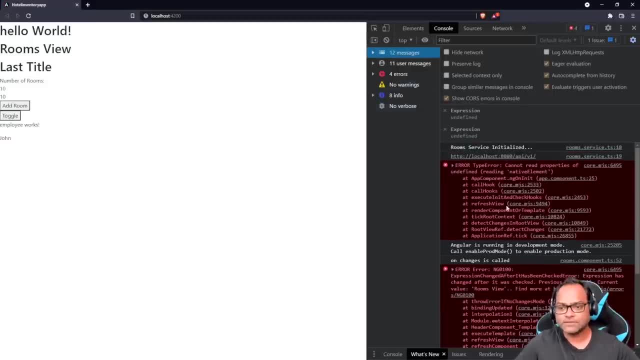 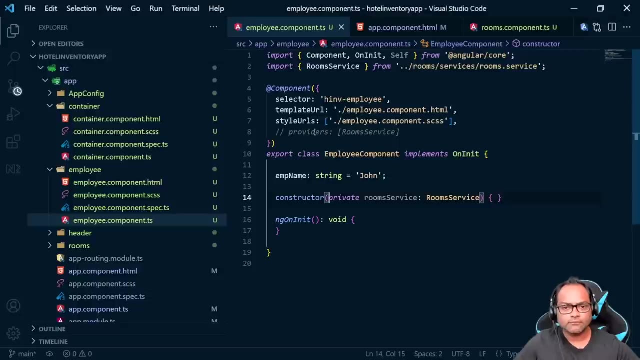 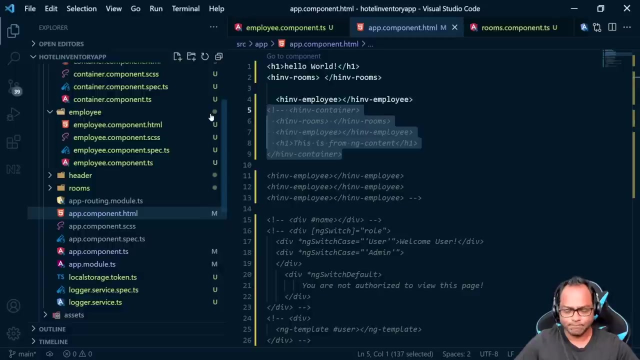 if you understand, if you remember right And let's go ahead and see now. OK, One more thing Which We missed is this container, right? So we have to uncomment this because we are not right now using container. 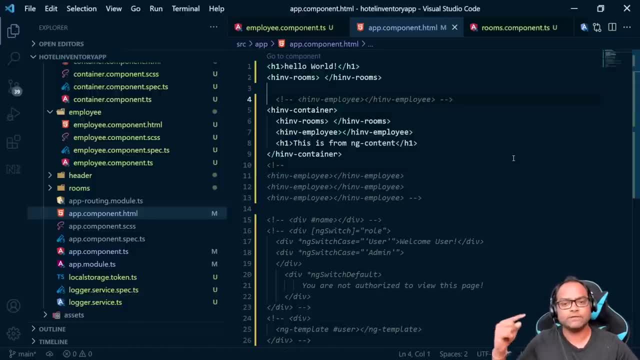 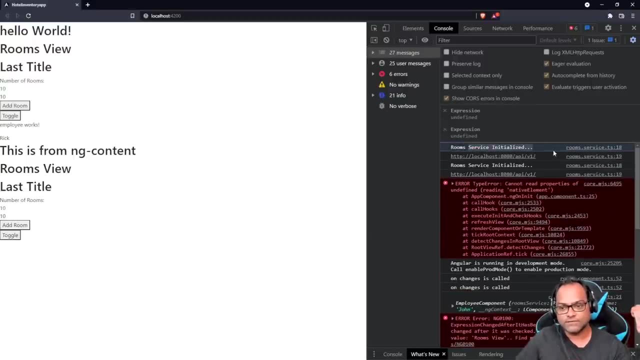 So I'll just do this, I'll comment this employee, And then I will just use the container And let's go ahead and see. So now you have two instances. So one instance is actually, which is, of course, global one. 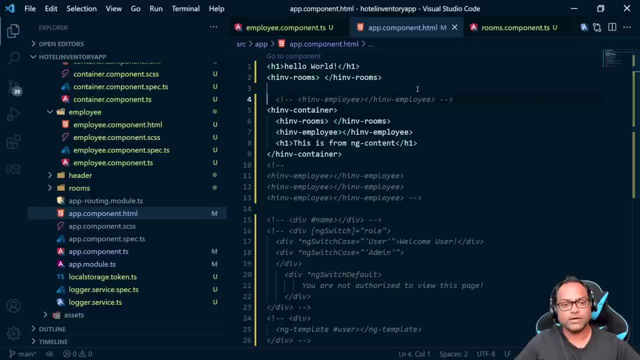 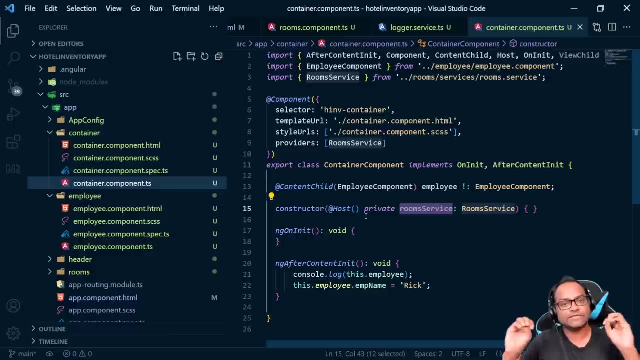 And another one is actually which is created by the container component. Now everything within container will start using the second instance, which is created by container. Also, we are saying this is host component, So actually none of the component which 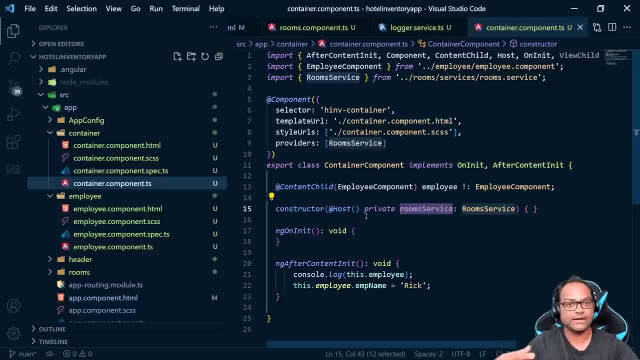 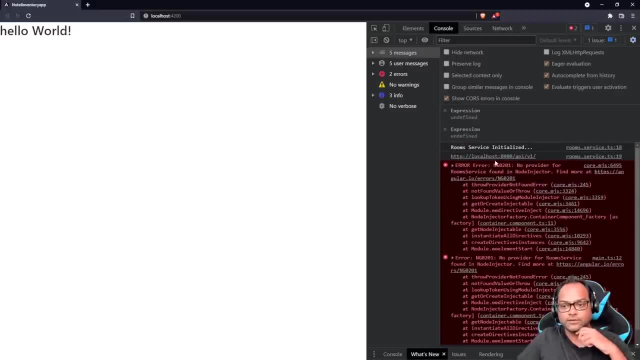 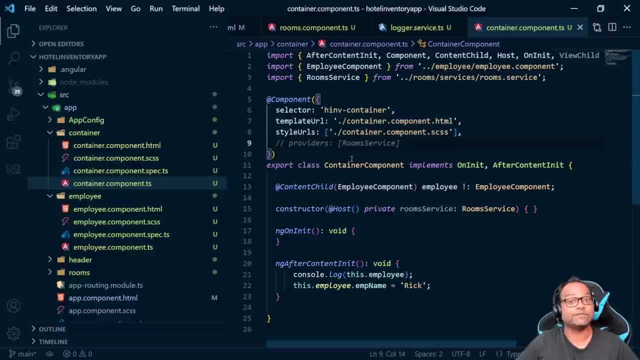 is loaded inside container will go above this particular level to look for this particular service instance. So if I remove this and try to run, you will start getting this: no provider for room service found in node injector. It will not go up. It will never go up and check with expand. 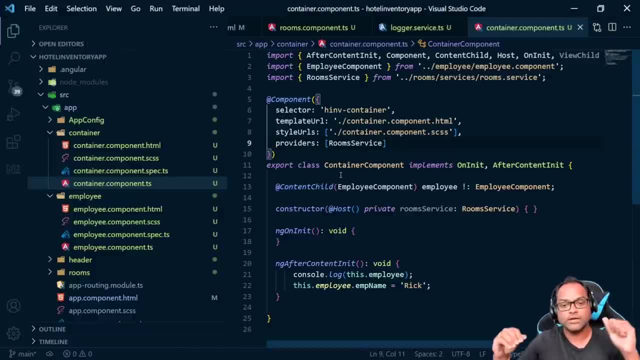 So this is what you can achieve using the host decorator. Remember most of the decorators you are not going to use daily, probably a few use cases where it may be useful. Skip self I have. as I said, it's not mandatory. 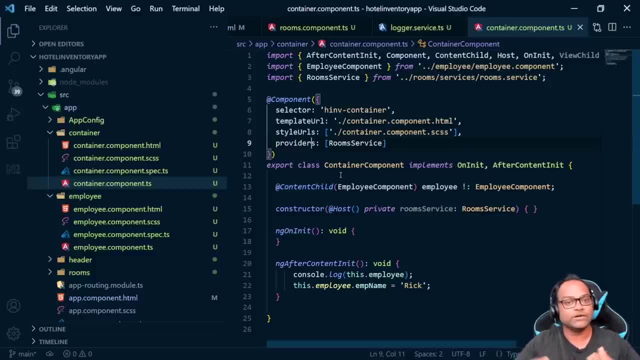 but you can use it As a loop filter is already pretty fast and you don't have to use it Self is really useful. Do use it in case you are using providers on the component itself, Not to actually avoid that, because loop filters is already. 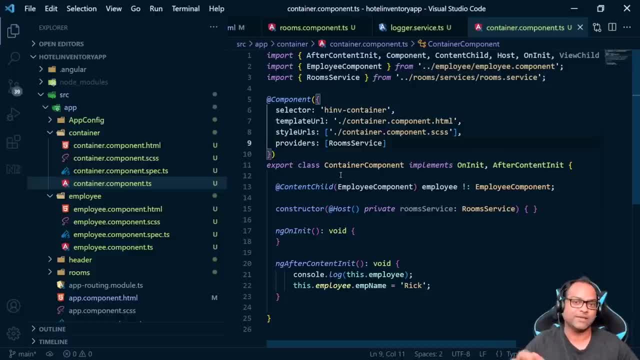 pretty powerful, but just to avoid the scenario which I mentioned, So sometimes by mistake while refactoring the code, we remove it. If you have it itself, it means OK. I actually really wanted to have this component, the service registered. 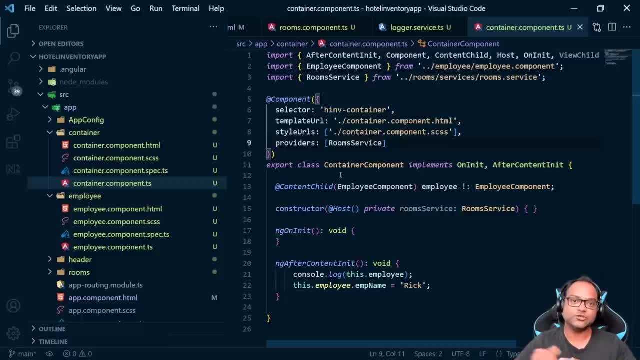 at this component level. And in case someone new comes in and joins your team and he figures out: OK, this provider is probably not useful and removes it, he'll start getting an error And probably he can read about self decorator. 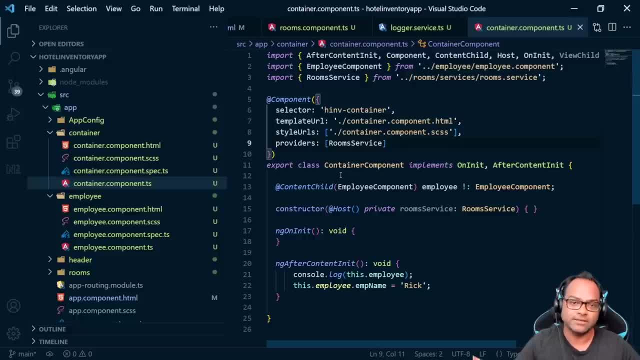 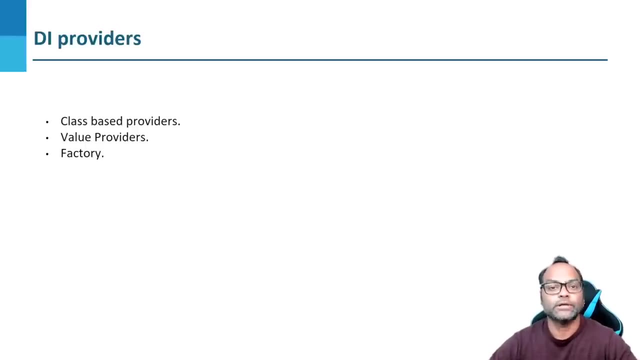 and what it is. Of course, documentation is a better way, but just in case, nothing is documented right. So this is all about the resolution modifiers And let's move on. In this video, we are going to talk about another type of service. 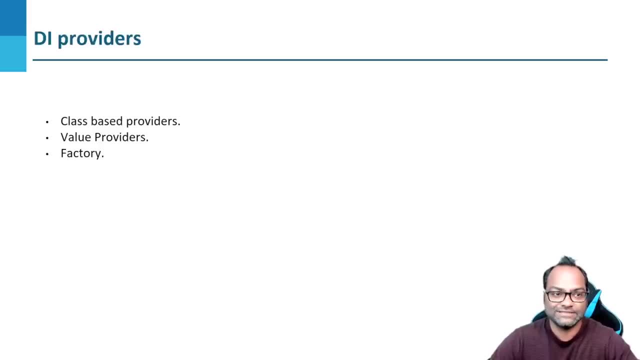 So, as you can see, there are actually three types of services which exist, So we have used the first type, which is class-based providers. So till now, whenever we used to do NG G service, we used to get a class with, of course. 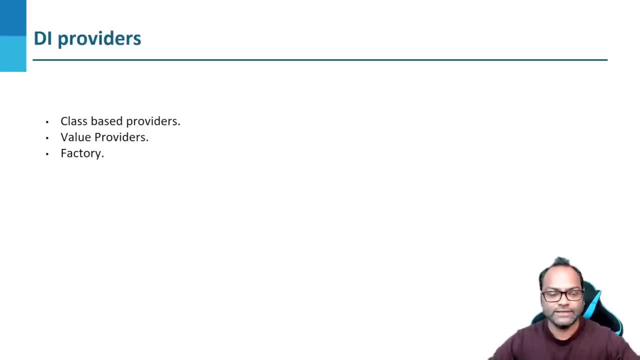 add-direct injectable decorator And we used to inject it and then use it. Let's go ahead and see where value providers can be useful. Value providers are like you can pass an object as a service And you might be wondering where that can be useful. 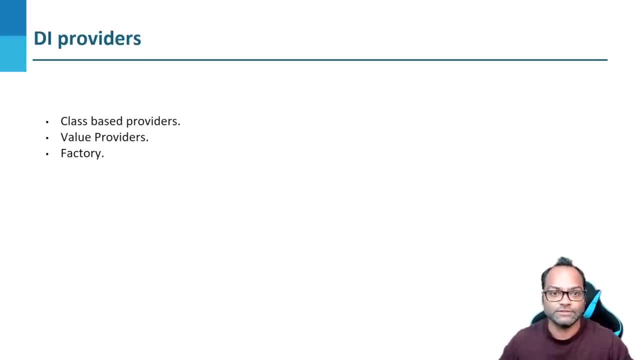 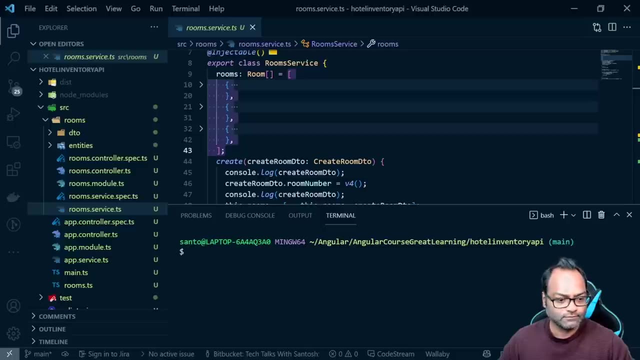 Why should I use object as a service? So let's go ahead and figure that out first. First let's see the use case and then we will create our service. So let's go back to our NG service And this is the code we have. 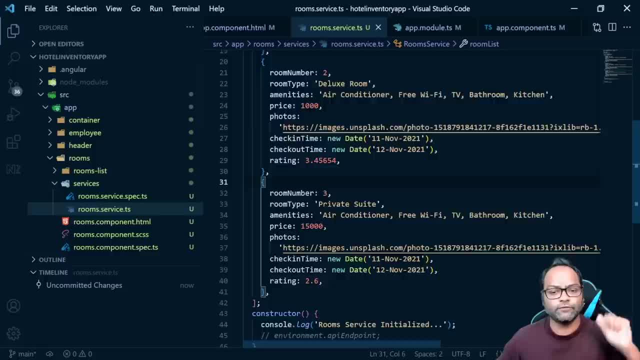 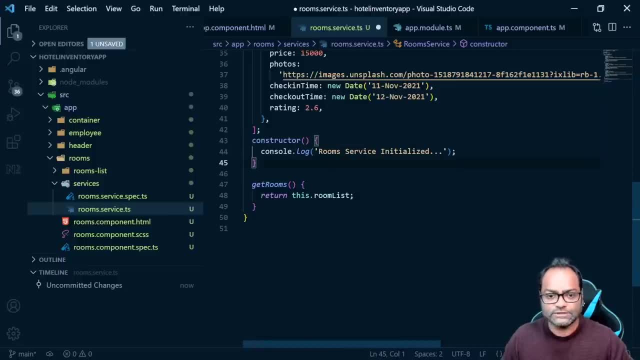 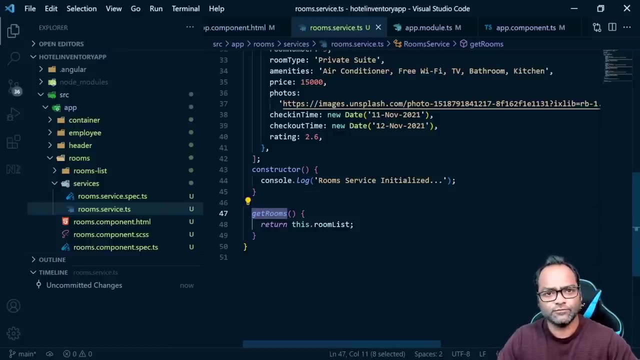 We have an constructor- and let me just remove this line- And we have a getRooms method, because this service does not do anything. I mean, this is a kind of static service with mock data. So this is a static service with mock data. 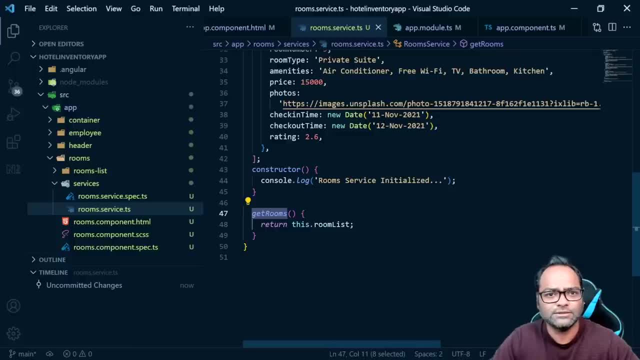 And this is a static service, So this is a static service, Right? Right? So this is a static service with mock data and it does nothing, Right? So we have just some dummy data which is available, and then we are getting this data. 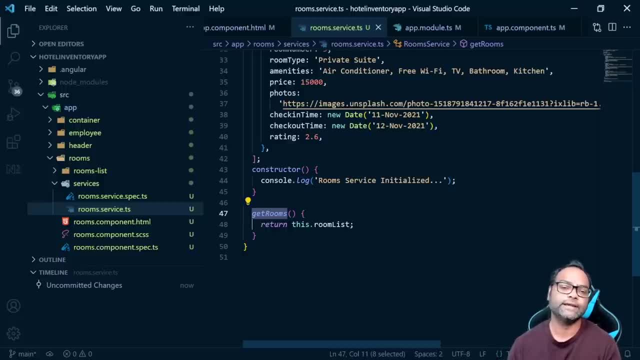 But once you create a real-time application, your data is going to come from, of course, an API, And for an API you need an endpoint. That's how APIs work, right? So what in that case? Let's see an example. 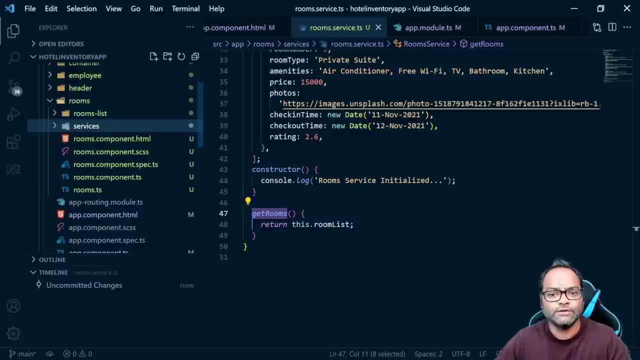 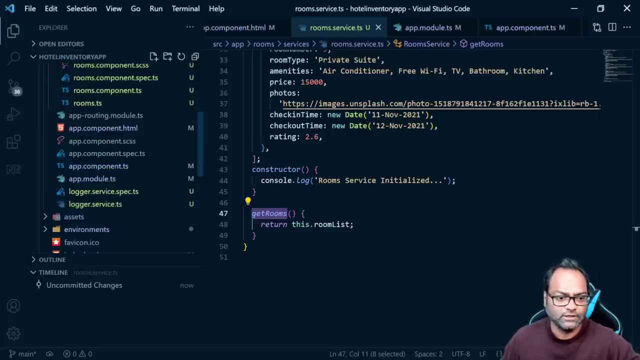 In case I have to access an API endpoint which will be used across my application, I mean in multiple services. what can I do? The first way: let me show you the simpler way which can be done. I can go to environment. 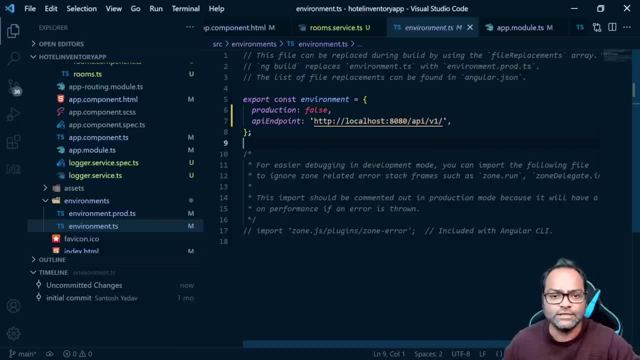 I have already added this endpoint here. So what I have done is, in environmentts, I have added a property called API endpoint, which is, of course, right now targets to localhost 8080 and some API slash v1.. So v1, version 1 of our API. 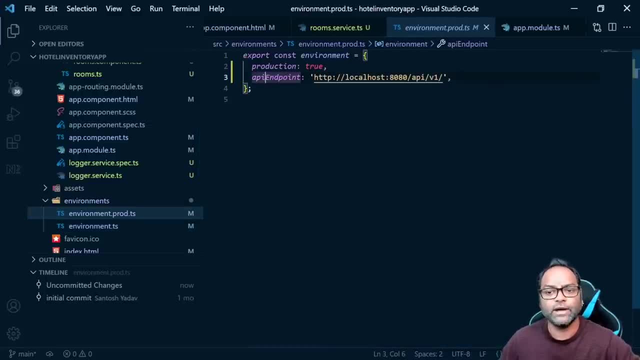 This API does not exist And I have to add the same configuration in productions so my build will not fail, Otherwise it will fail. So remember, in case you have multiple environment files, whenever you change into your environmentts, make sure you make the same change into every environmentts. 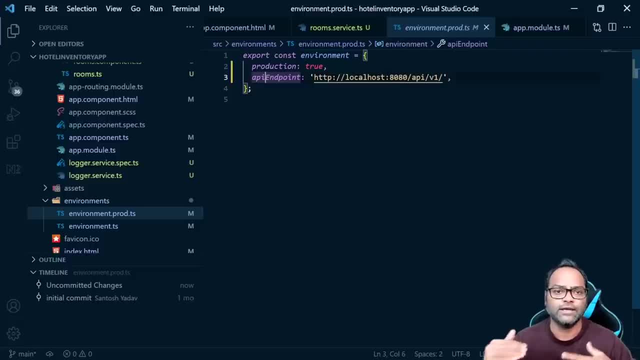 file which is available. For example, I can have one for staging, I can have one for UAT And, of course, two are required, which is environmentts and prod. We will discuss this later on, while deploying our production application, how we can change the settings. 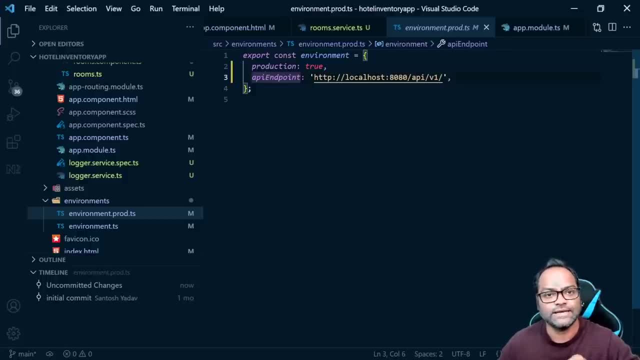 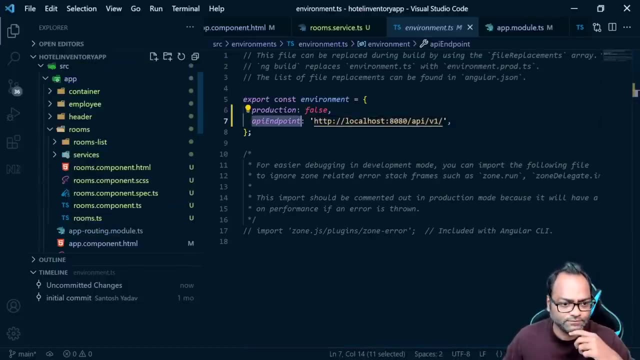 But right now, just remember. So whenever you add something, just make sure that it is added to all the environment files And in case I want to access this API endpoint inside my service, how I can do that, Let's go to servicets. 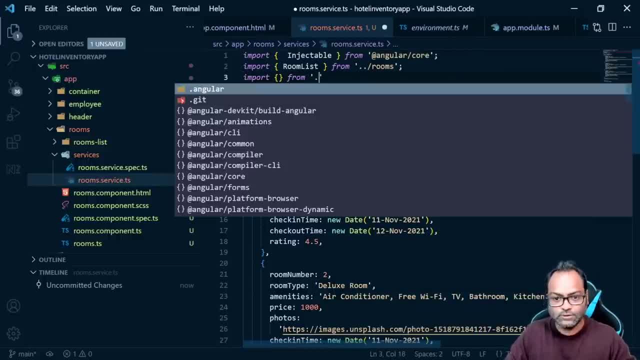 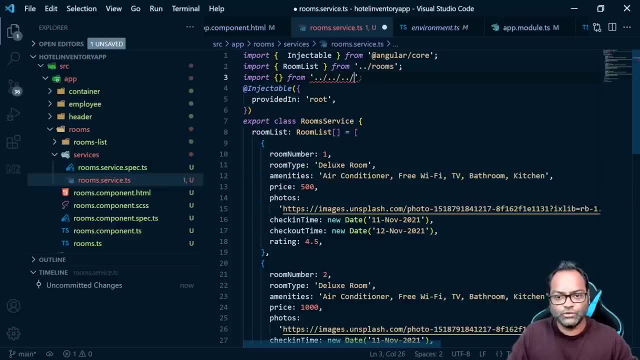 And I can import from dot dot slash, dot, dot slash, dot dot slash until I reach to environment And then I can say The environment file And then I can just access the property So environment, And then I can use this environment anywhere. 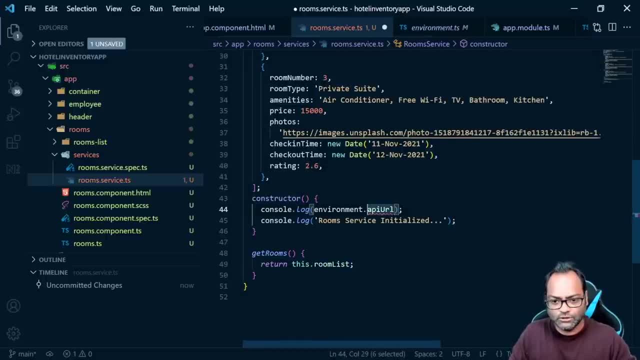 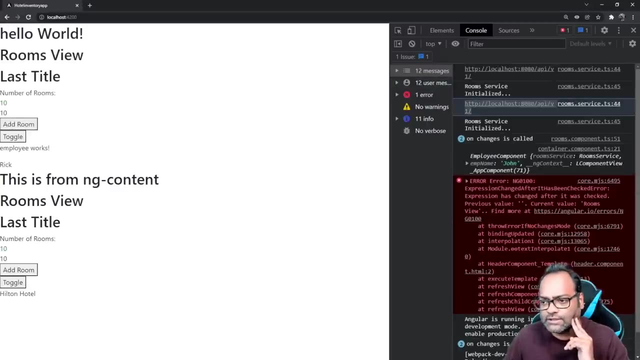 So I can just say here: console dot log environment dot API endpoint, And let's save this and see, And you have this URL available. So here you can see service line number 18.. Sorry, 44. And we have this API endpoint which. 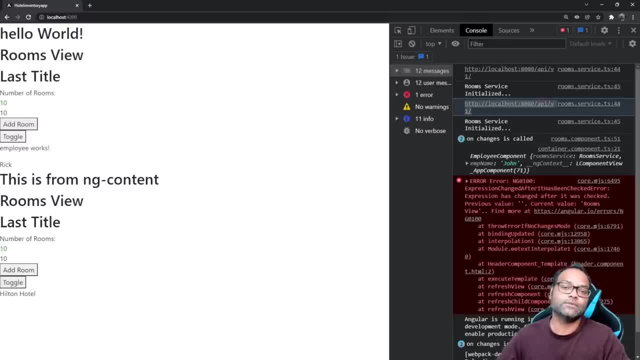 is available in our config file. But what we are talking about here is we are saying this URL will be used at multiple services. What, in that case? Just think about your import. I mean it will be everywhere. I have to give entire path. 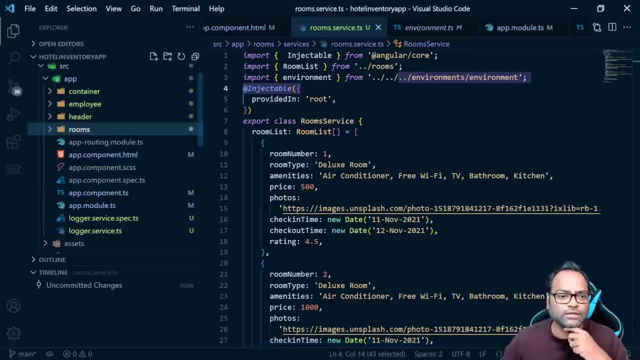 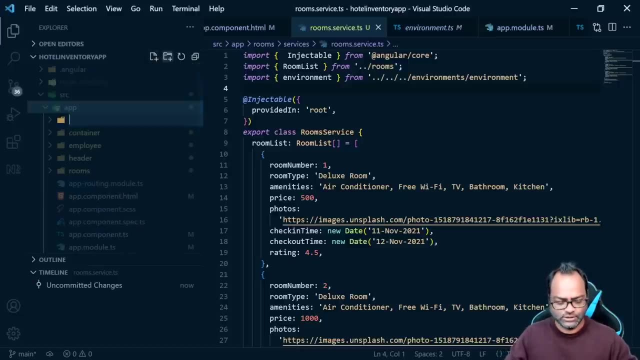 How I can avoid this. So this is where the value providers come really handy, And we are going to see two examples. So first let's see how we can actually deal with these objects, Right? So what I'm going to do is I'm going to create a folder. 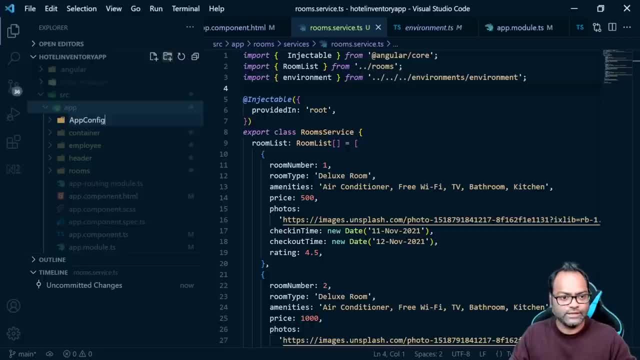 I'll call this as a config, So it will contain some services related to application configuration. So the first thing which I'm going to do is I'm going to create a service. So let's see how we can create a value provider, Right. 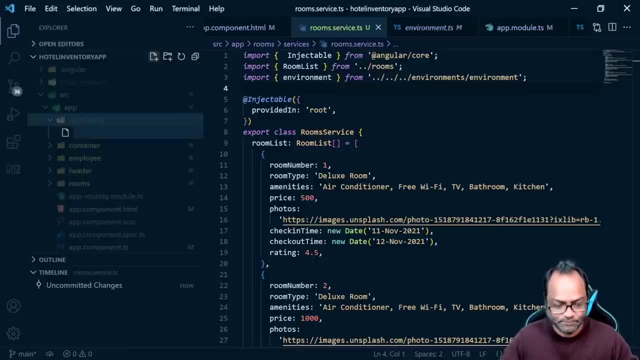 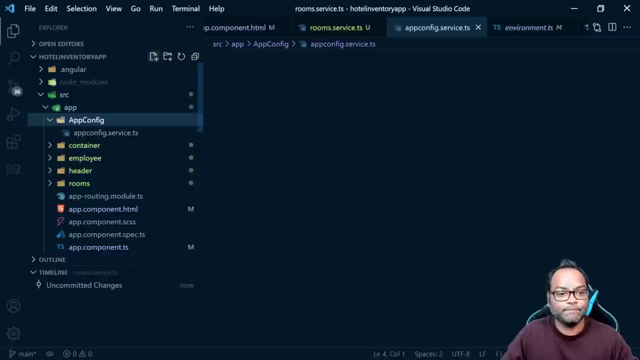 I'm going to call it as a service because it is. We are going to actually inject it, So I'll call it as a config, Dot Service, Dot These. If you're wondering why I'm typing it, because of course there is no command for it. 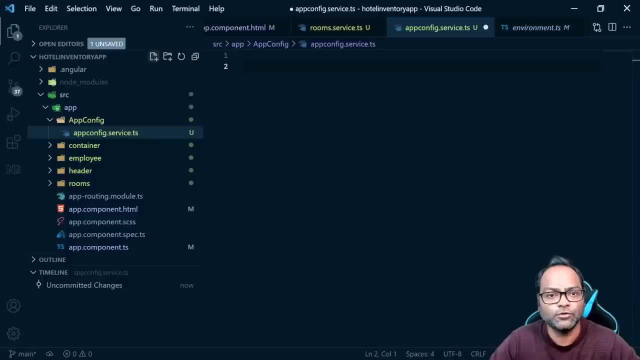 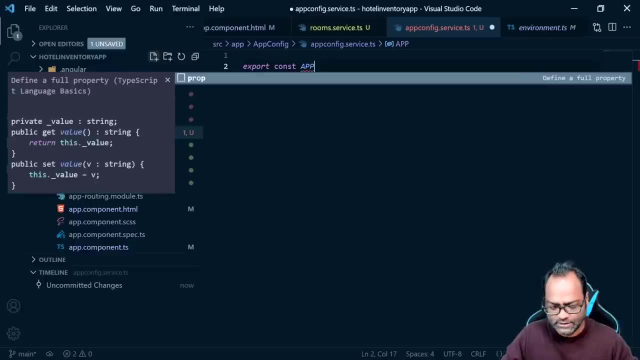 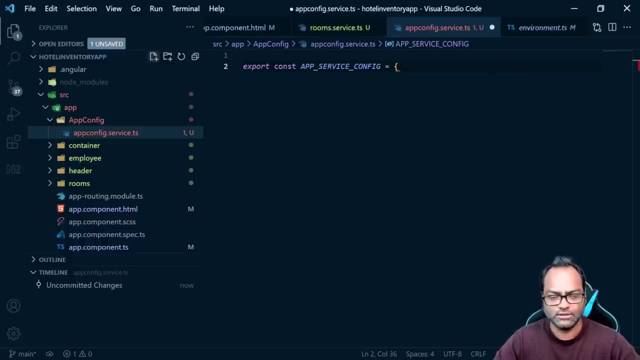 You have to do it manually. So the first thing which we are going to do is we are going to create Export constant and I'll call it as a service. It depends, I mean, if you see I'm using capital letters, but it's okay. 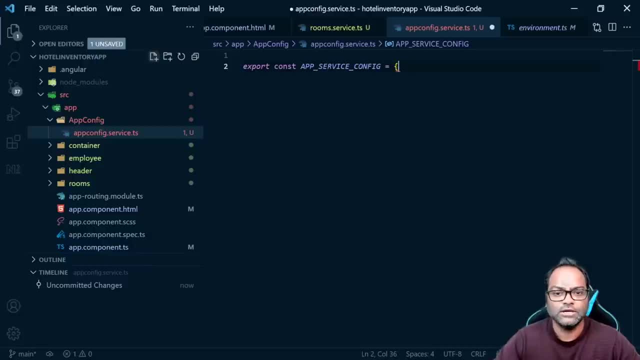 Even though you don't use capital letters. that's absolutely fine, because I generally we have an habit of mentioning const as capitals, but it's not mandatory, So choose whatever you're comfortable with. And then what I have to do is I have to create a new injection token. 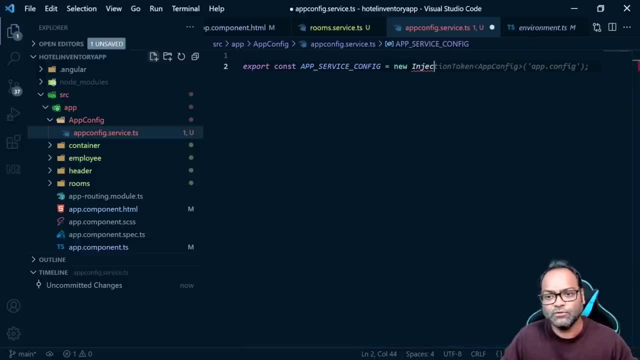 So I'll say new injection token, And you can see I'm using something known as GitHub Copilot. That's why I'm getting this autocomplete. So I'm going to use it And let's import injection token from Angular core And then this is app config. 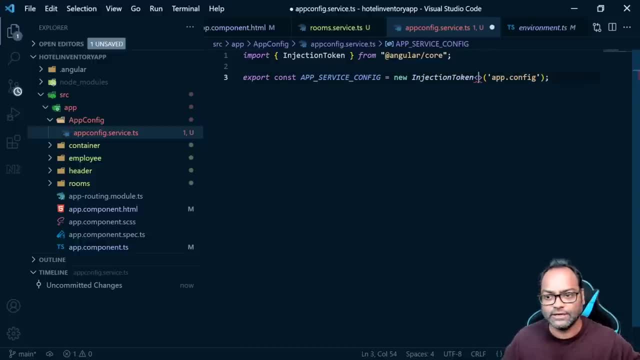 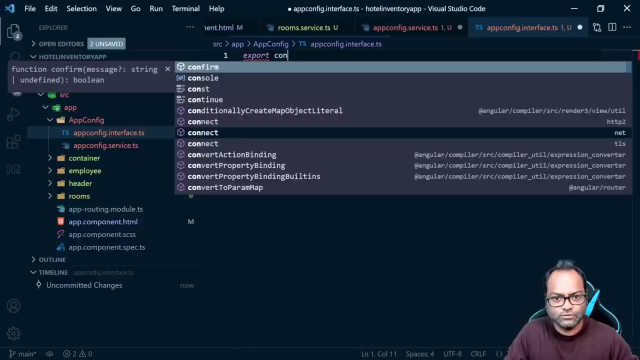 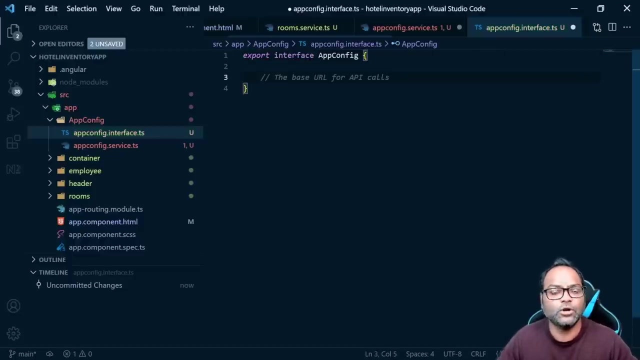 Right, This is actually an interface We are going to create, So let's go ahead and create that. I'll create an interface. Let's call it as appconfiginterfacethis, And let's do. Let's create an interface, And you can mention all the properties which belongs to your app configuration. 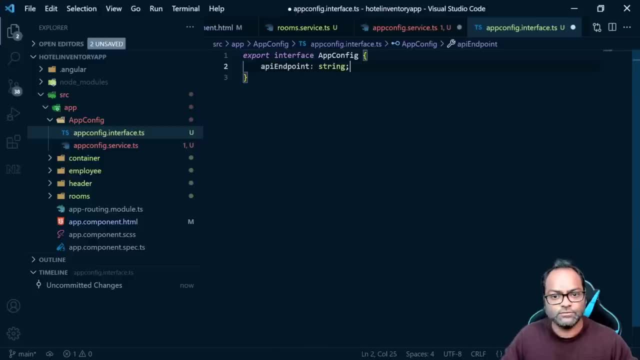 And so, right now, what we are going to do is I'm going to use API endpoint. This is the only property We have, But in case you have more, just go ahead and add all the properties here. Now, here I can just use the same interface which we have created. 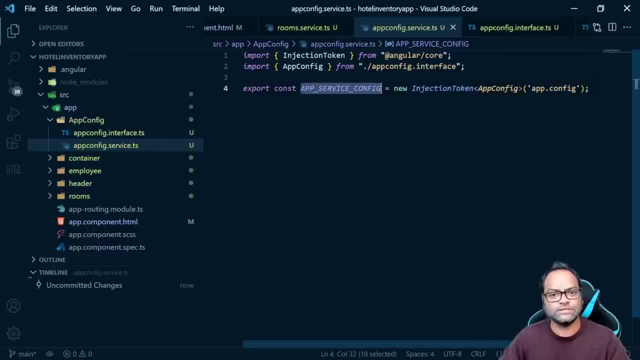 And let's import it. So this becomes my service. This is, this is the service we are going to use, But we also need the data. So by value providers means I'm going to provide some value. Let's go ahead and create a value. 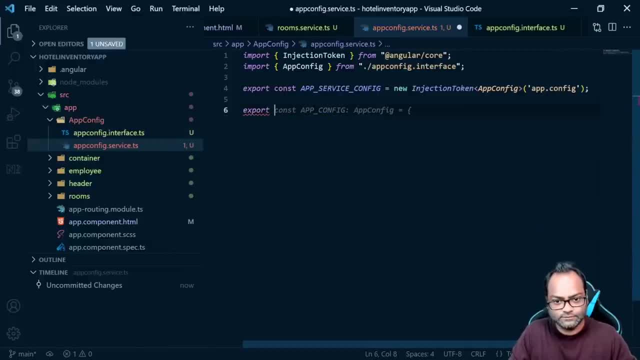 So I'm going to create another constant And I'm going to call it as appconfiginterfacethis, And let's provide the value. So here I can say API endpoint, because this is the property we have here, And then we have to provide the value. 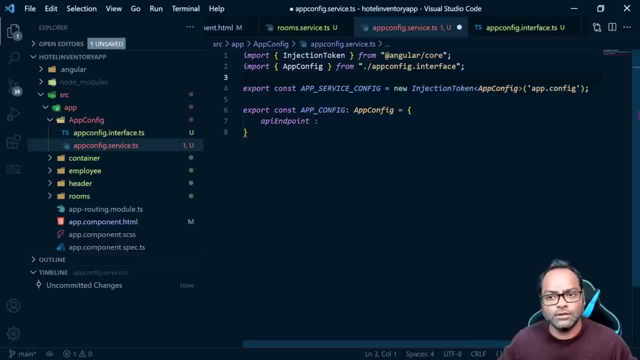 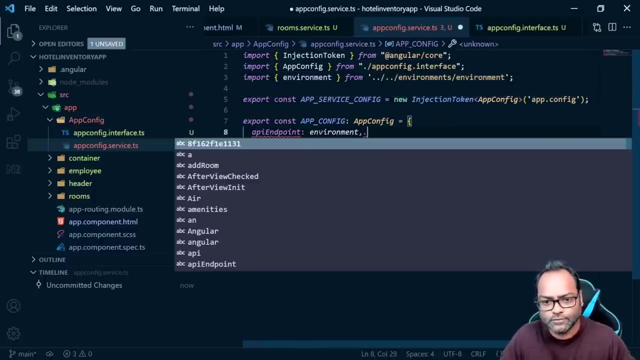 Now what we can do is we can import our environmentts file here And slash dot dot. slash environment, slash environment And take the property which we need. So we are going to need environment dot API endpoint, And now I have to do it at only one place. 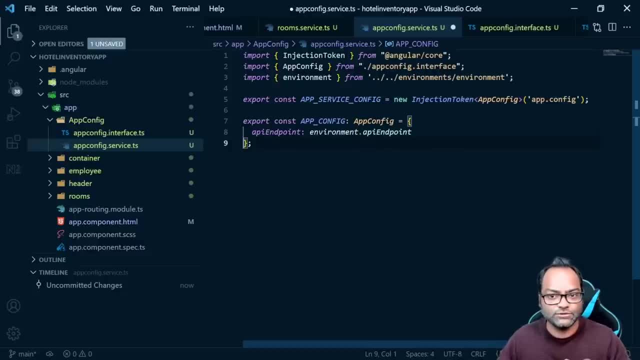 I don't have to repeat this: inside edge and every service, So we don't have to do it. So now this is done, So we have our service ready. We have- Sorry, We have our service ready. We are, We have our value ready. 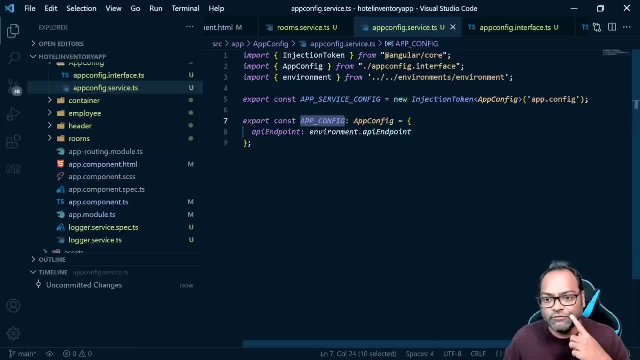 Now let's see how to register this particular service, because we have not done this Right. We don't have anything called here, called provided in. So let's see, Let's see how to do it, So we can go to app module. 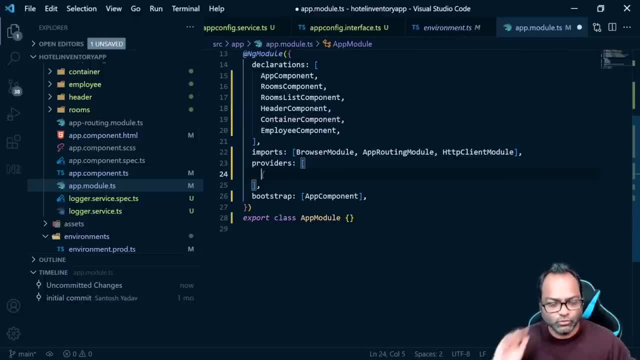 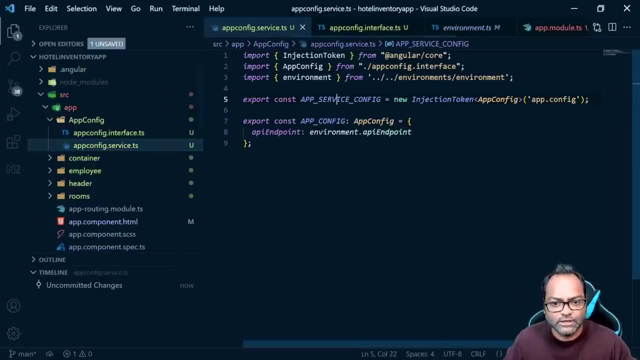 And you know that you can see this: providers here. This is where you can register your service. So you can say provide- Sorry, It will be an object. So I can say provide, And here I'm going to say provide this particular service. 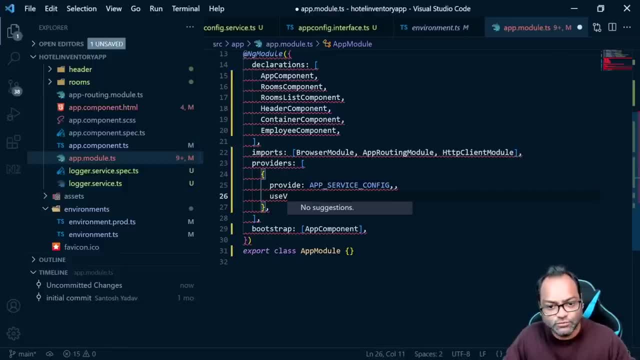 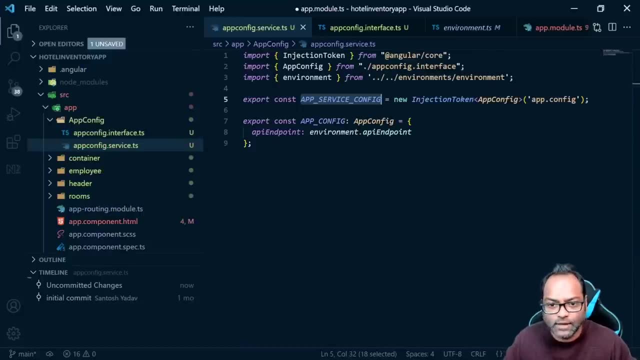 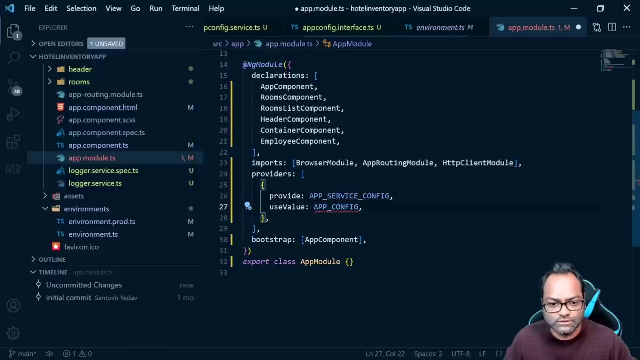 And I'm going to use a property called use value And inside value. I'm going to say: this is the value And let's import both. So I'll just Done So we have. what we have done so far is we have created a value provider. 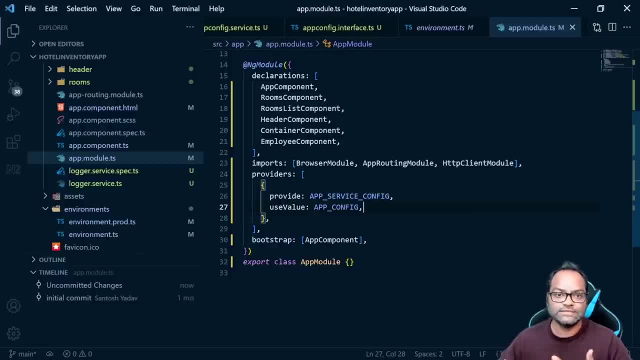 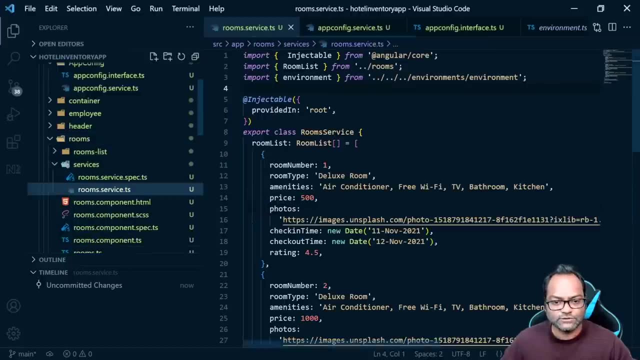 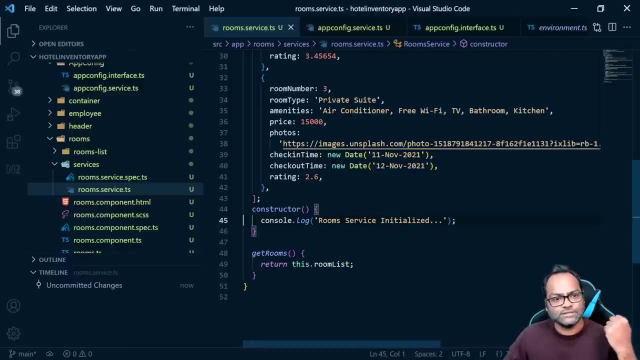 We have registered that value provider. Now the next step is to use this provider. Let's do that. I'm going to go back to RoomServicets. Remove this, And now we need to access the URL from that particular service which we have created. 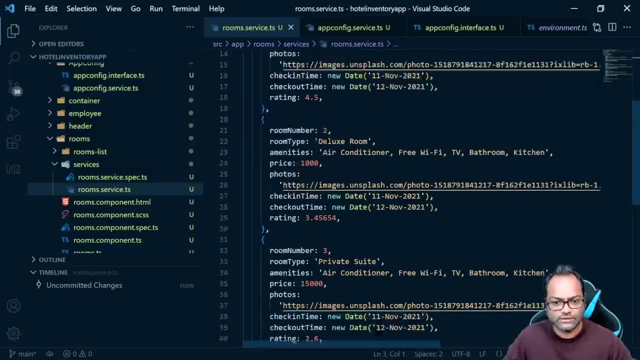 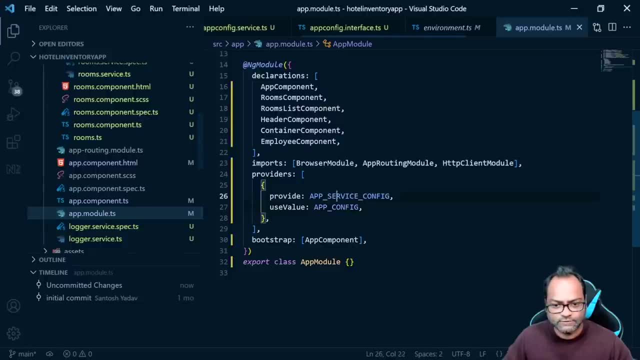 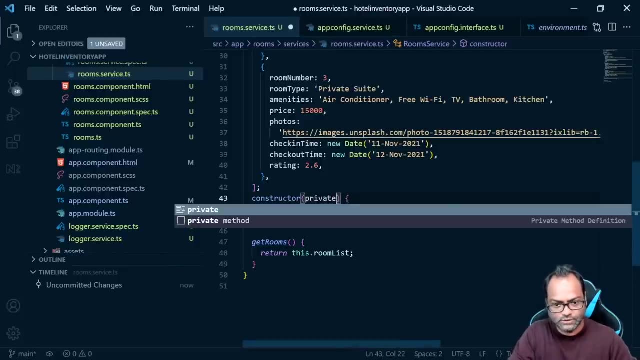 So we know, we know how to inject a service, So let's try that Constructor, This here, And Our service name is AppServiceConfig. So If I do this- And you can see I cannot Right- Even my intelligence says it is not something which can be recognized. 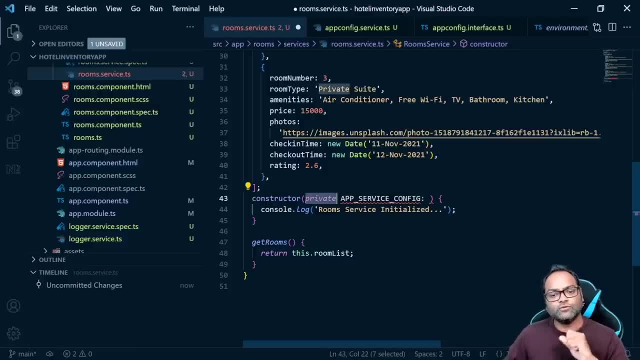 What is this? So the way to use the value providers is you have to use something known as inject decorator, And then you will pass your service here, AppServiceConfig. So let's import. Now you can see it. It is giving me the path somehow. 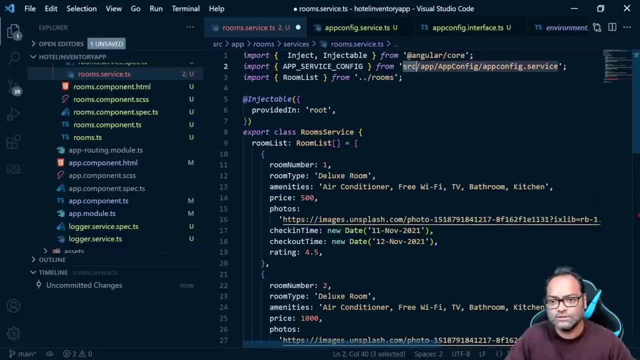 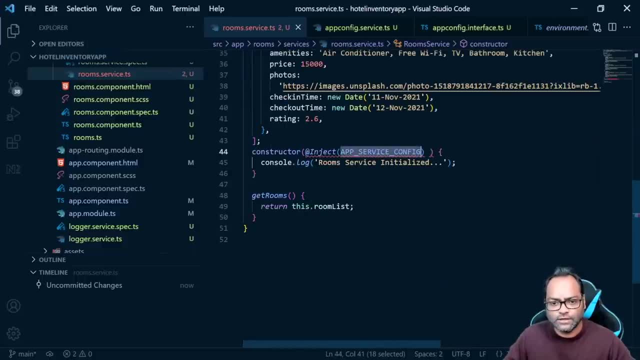 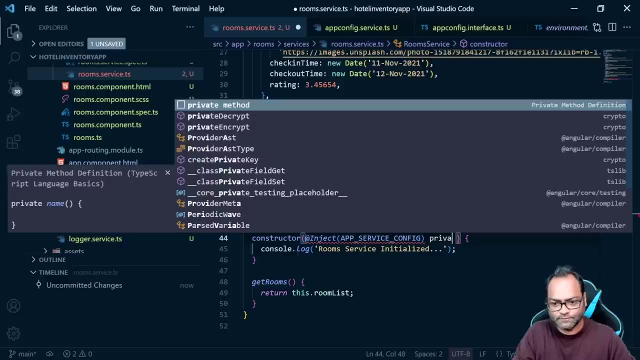 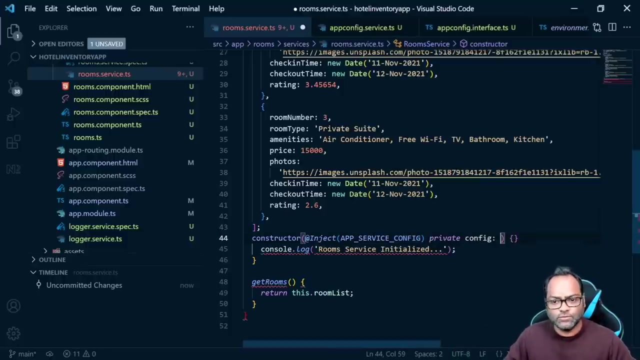 Let's change this. It should not be SRC. So we have our app service we have to use at direct inject decorator, And now I can say private, So I'll call it as config, And Here we don't have to use type any, because we also know the type. 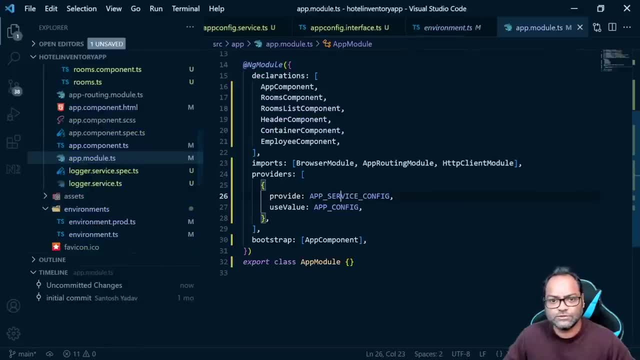 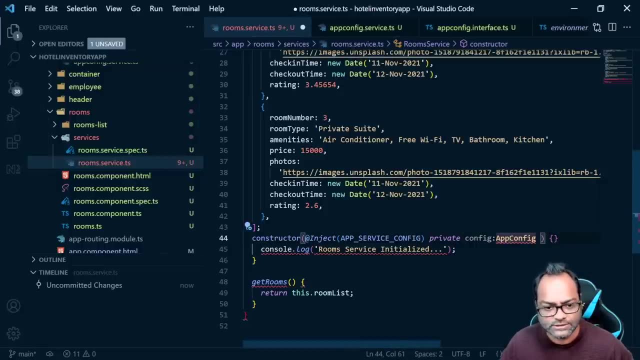 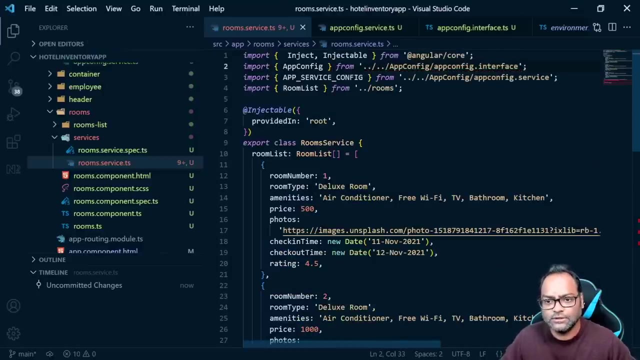 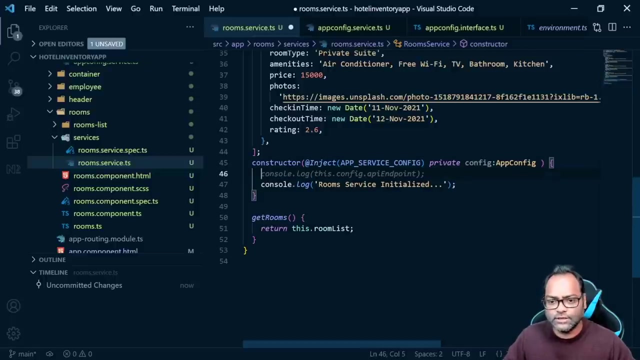 So let's go back to the service. This is the type AppConfig, So we can use this particular type here, So we get proper intelligence Right. I mean even the typings. And again, this is. This is Now let's try to access the same API endpoint by using this particular service. 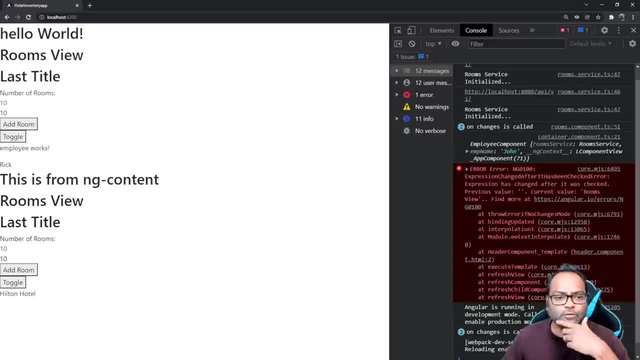 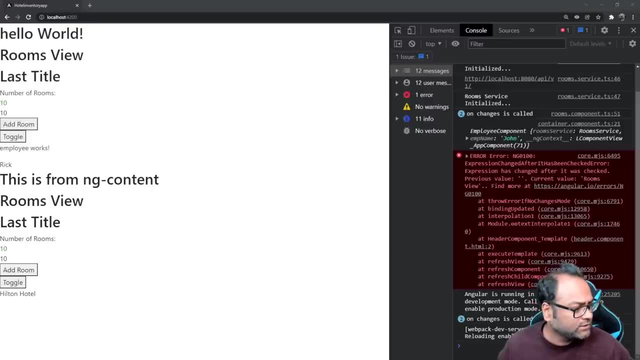 So let's save this, Go back to the code base and Go back to the URL And let's see if it is compiled. It is compiled, So let's see, And We have room service initialized here And this is your endpoint. 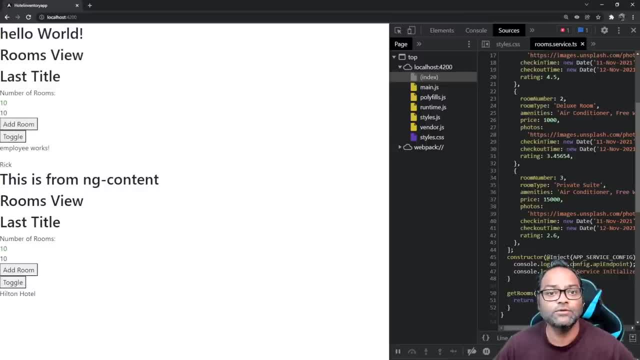 So you can see line number 46.. Now we are actually getting this value from a value provider rather than actually directly accessing environment, A value from environment. What we are doing is we are, we have created an Injection token, or we have created a value provider, and then we are using it. 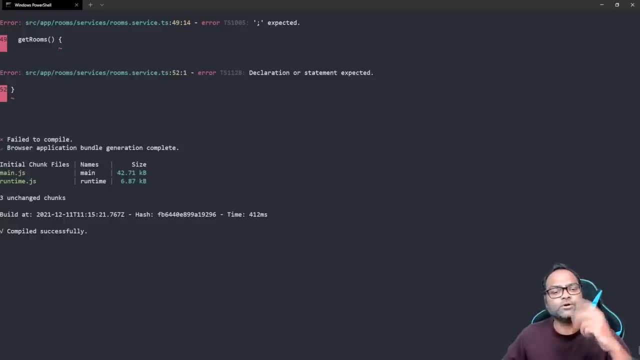 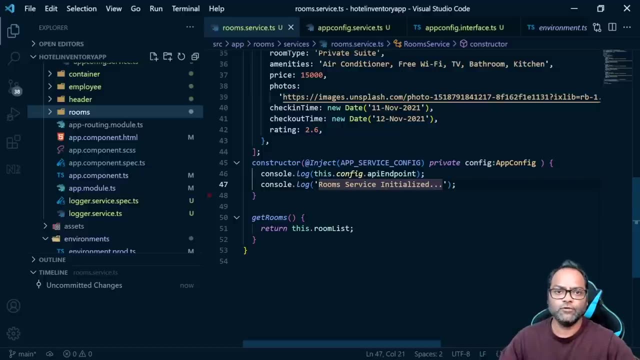 So this is the way you should be doing that. Now let's talk about the second use case. So if you have, By learning JavaScript, you might have seen some APIs right. I mean, you may have seen Windows. We have local storage, session storage. 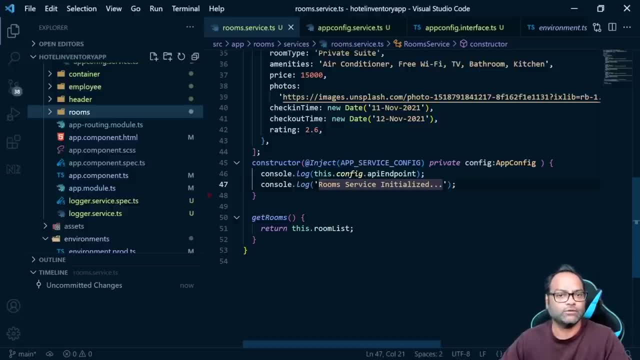 What in case? I want to use those inside Angular? Of course you can, because of course that's JavaScript And Angular at the end gives you JavaScript as an output Right And it's a front end And every JavaScript code is a valid TypeScript code. 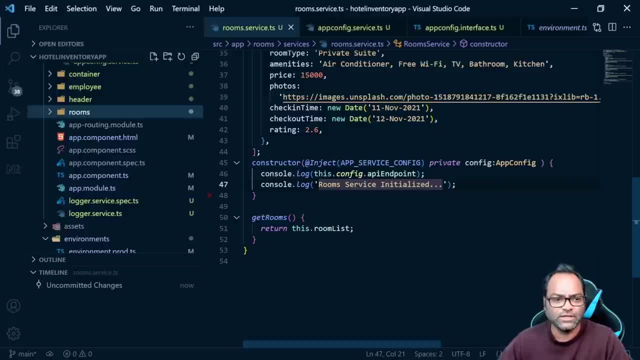 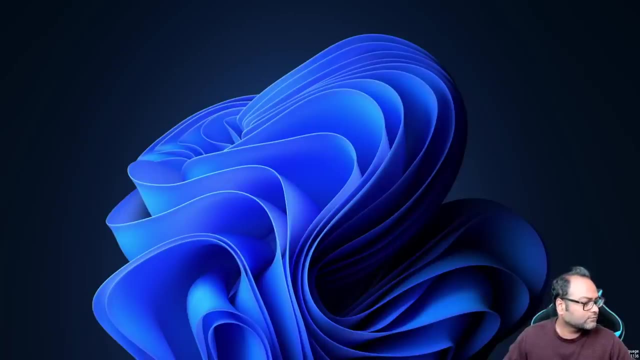 So you can use that, But there are some ways, So there is, there is a way to use it. So to do that, I will take an example where we will use the local storage service. So, So, So, So So. 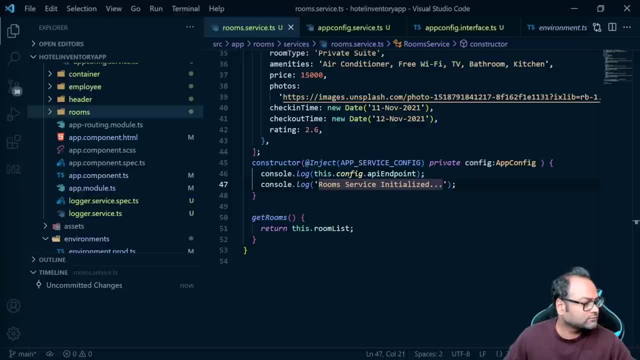 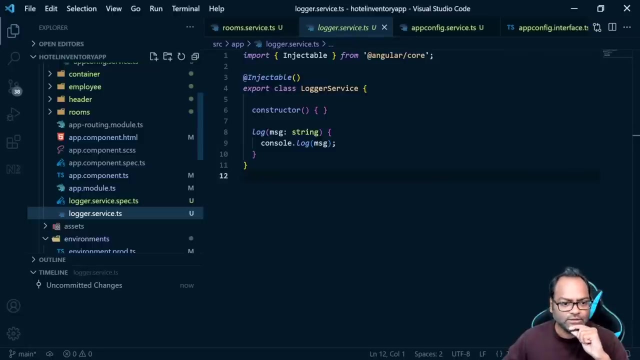 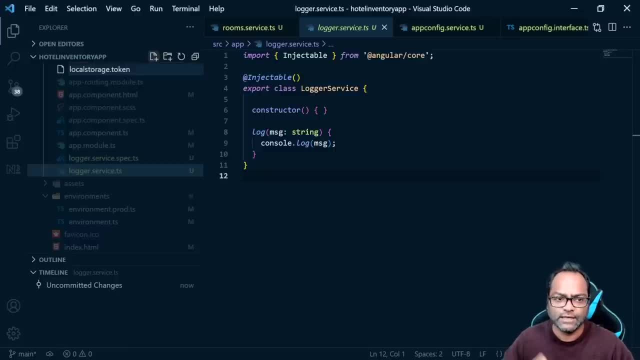 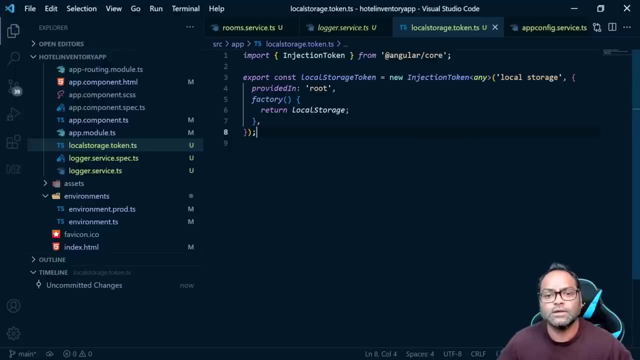 Remember, any JavaScript API which you have seen can be used in this way. Yeah, Yeah, Yeah, in this way, and i'll just copy some code. so here, what we are doing is we, of course, we are creating an injection token, we are using provided in root, here, because i want to make sure that this: 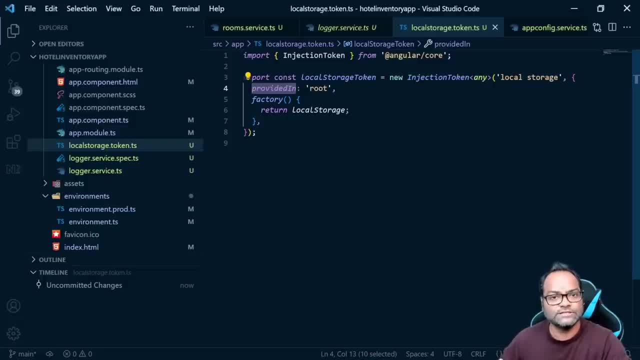 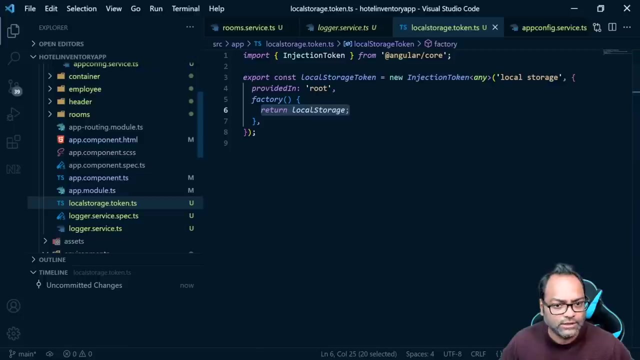 particular service is trace checkable and if no one is using it, it the code can be removed. it and i'm calling a factory function to return a new instance of local storage. that's what we are doing here. we don't have to register this service directly anywhere. so, uh, let's see how we can use. 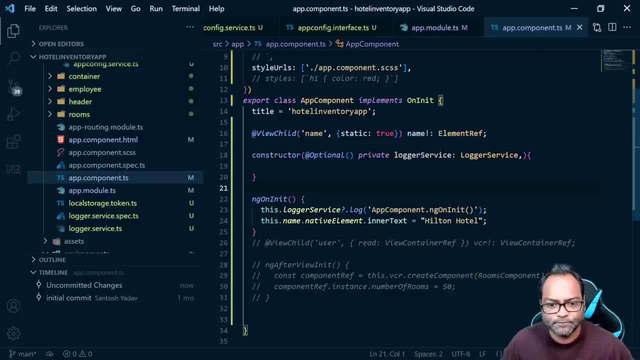 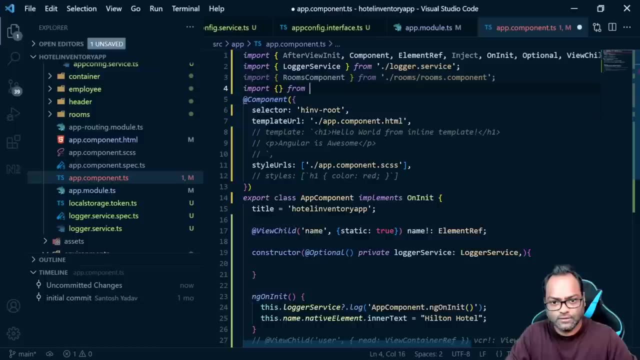 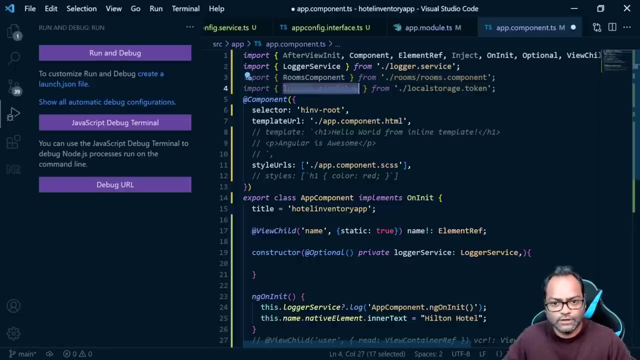 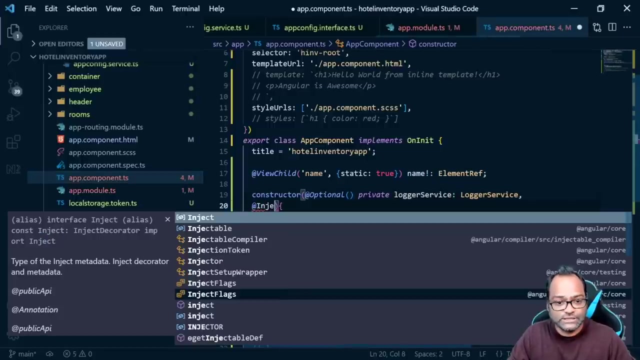 it. so i'll go to app componentts and here let's see: uh, we will inject a circle import from dot, dot slash- okay, dot slash, local storage token, and we will we need to use inject, right, and then we'll call our local storage token, which is: 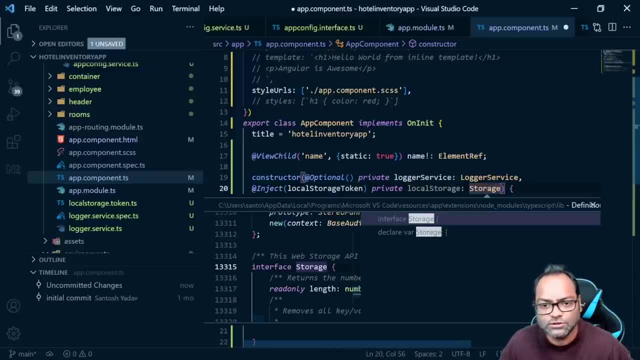 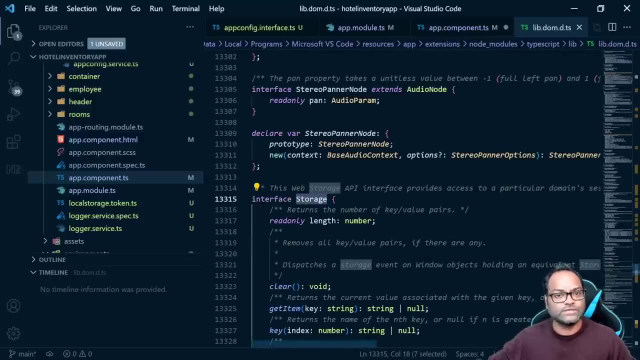 type of local storage and you can also give type storage. so this is any uh, this is actually uh the type for your. let's see, yeah, this type for your uh storage api, which is which, again, which exist in browser, Actually TypeScript, all 3D has type definition file. 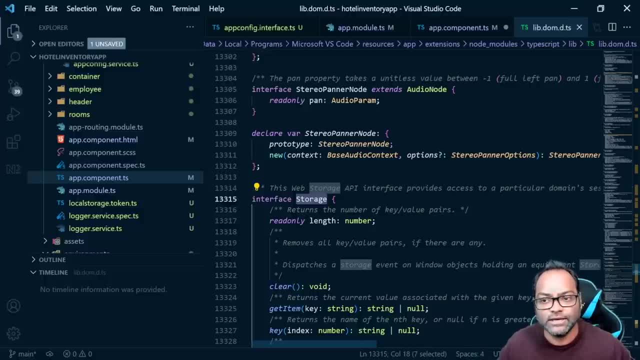 for most of the web APIs or JavaScript based APIs which we use generally. It's a file called libdomts, because it's all related to DOM right, So here we can use it. in case you get any error while compiling, just move it to any. 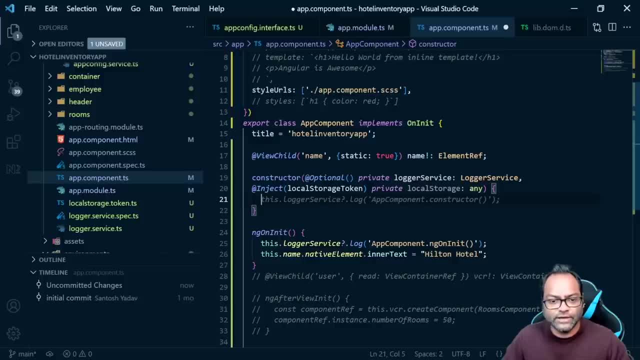 That's subsequently fine. And once this is done, let's go ahead and add something to local storage. So to do that, I'll just add one value. So let's add on ng, on init, let's add this value into our local storage. 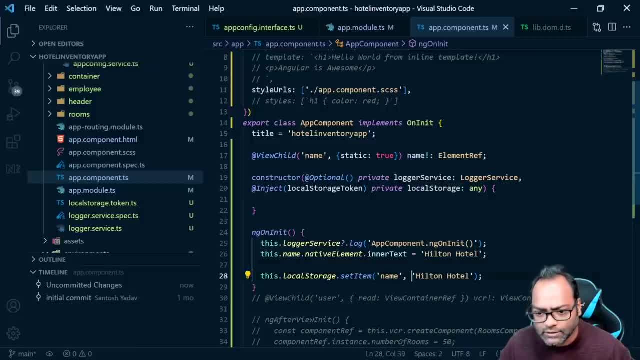 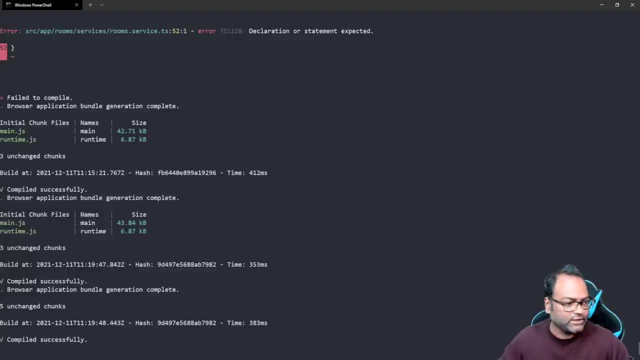 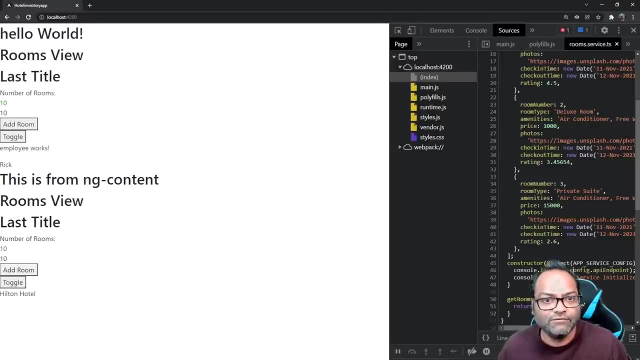 So I'm adding a variable called name and the value is: Let's see. this value will be added once our app is loaded, right, Because it's on ng, on init, on our root component. let's go ahead and see. so this is, uh, where you can verify local storage. 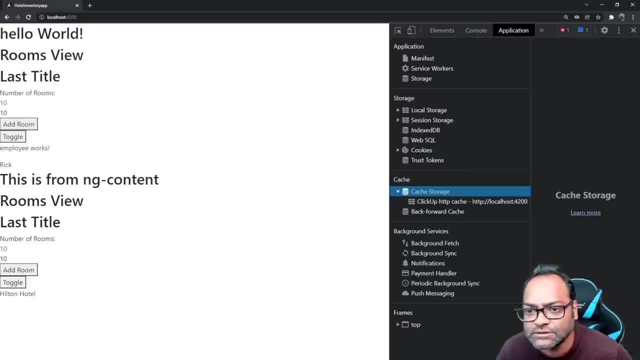 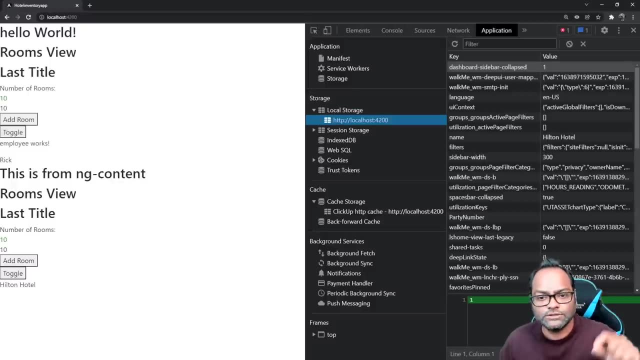 so here you can go to your application and just see local storage, localhost 4200. right, so, because our application is right now running on localhost 4200, you can see this value. name: delta nodule: yep. so this is. this is where your value will be available. don't try to add anything, uh, which is secure, to your local storage. this is. 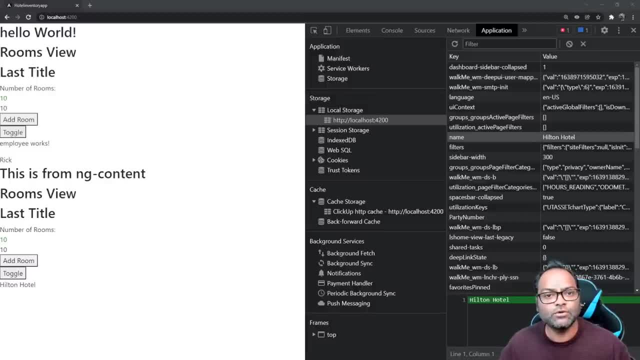 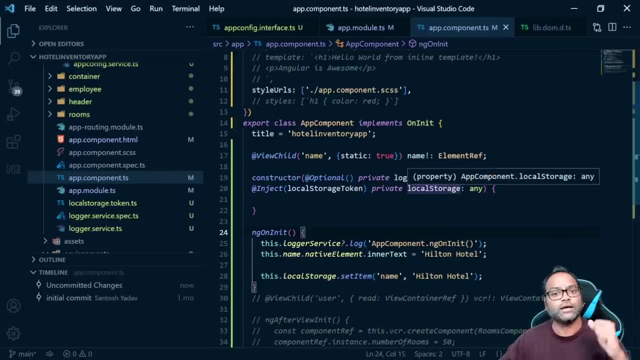 just an example how you can use local storage. in similar way, you can also use session storage. so, in case i, in case you want to use look suggestion storage inside your angular application rather than directly using it, try to create an injection token like this which, like the one which 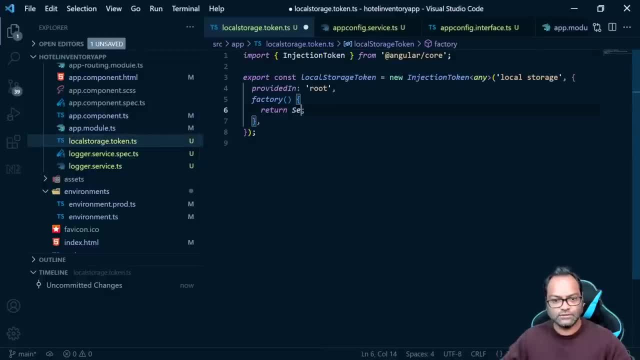 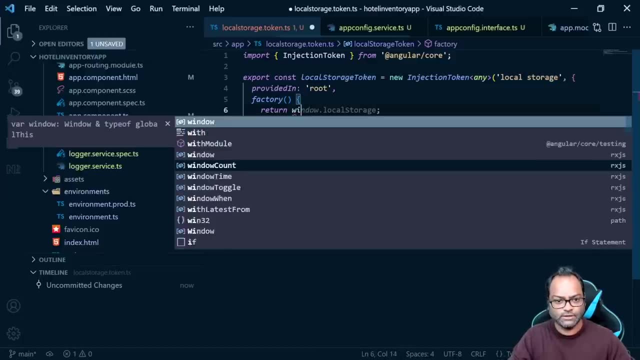 we have created for local storage. the only difference would be session storage right, and even you can use other apis, for example uh window dot, for example, in case you want to use uh location right. so, rather than actually injecting location directly, which is uh, or accessing location directly, which is possible- yes, of course it is possible- try to use it open so you can use location. 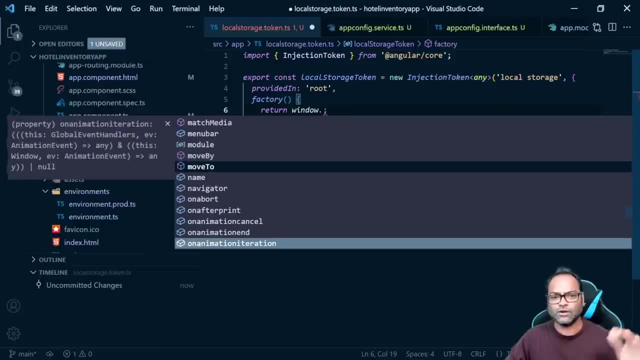 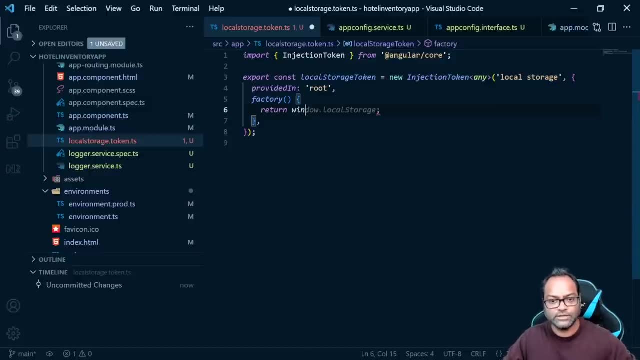 menu bar there are navigator. there are a lot of apis which access, right, i mean you can- all you, you can use all those apis as a token here rather than actually directly using inside your code base. in case you come across any existing code base which is not following this, try to refactor. 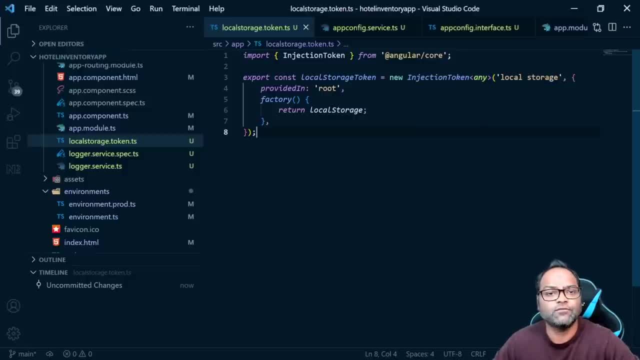 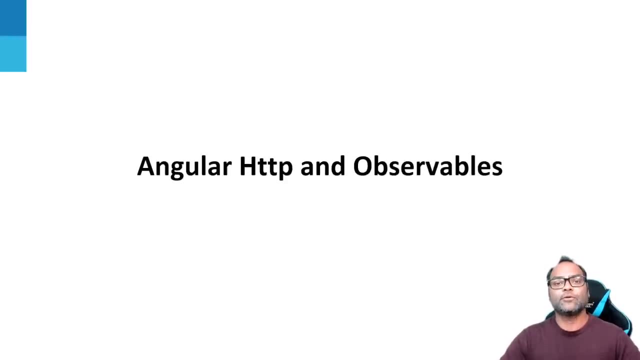 i mean, you will learn something new. so this is it from value providers. in this video we are going to talk about angular http and observables. this is really important to understand because in your enterprise applications, what you are going to do is most of the time you 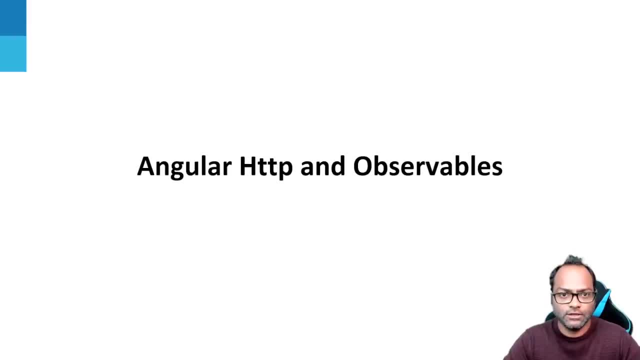 will be interacting with the apis. so this is what we are going to learn here: how to interact with your apis, how to handle the http uh calls and how to do different http calls. so let's go ahead and see uh the agenda for this particular video. so we will, of course, go through the introduction, then we will set up. 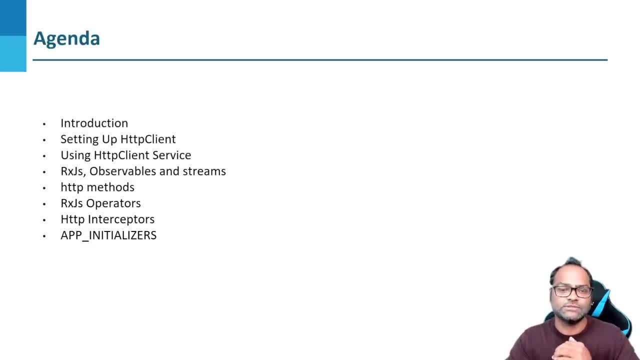 the http client. we will use the http client service, which is which will be used to make those api calls. we'll talk about rxjs. we'll talk about observables and streams. we'll see different http methods which exist. we'll see some examples of rxjs operators. 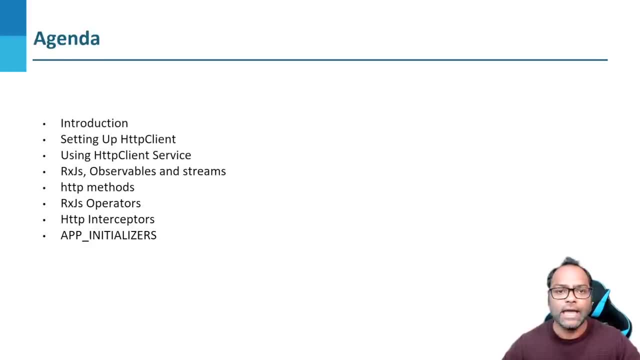 and then we'll see http interceptors and at the end we will see app. at the end we will see app initializer. so let's go ahead and see. uh, why, uh, this angular http is important. so in enterprise application, as i said, you will be interacting with apis in javascript. you might have used 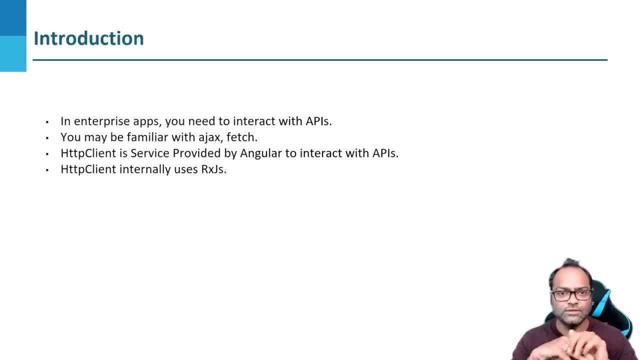 ajax or fetch. if you have never used it, that's absolutely fine. that's, those are the low level apis which is available inside your browser. http client is is the service which we are going to use to interact with our apis, and http client internally uses rxjs. so what is rxjs? of course, 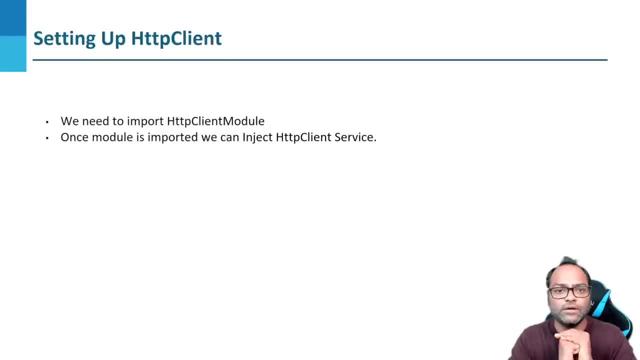 we will see that, but let's go ahead and start with setting up our http client. to use the functionality provided by http client to interact with your apis, we need to do some configuration, so let's go through that, those steps. the first step is we have to use something called http. 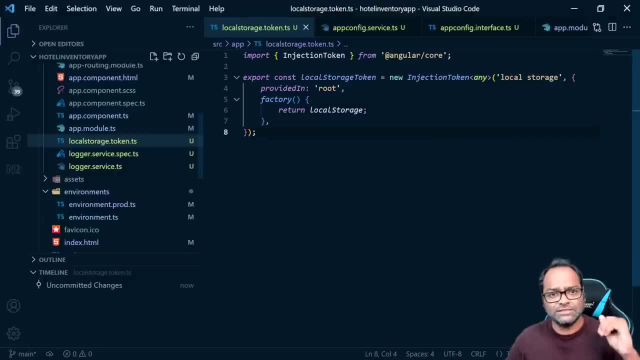 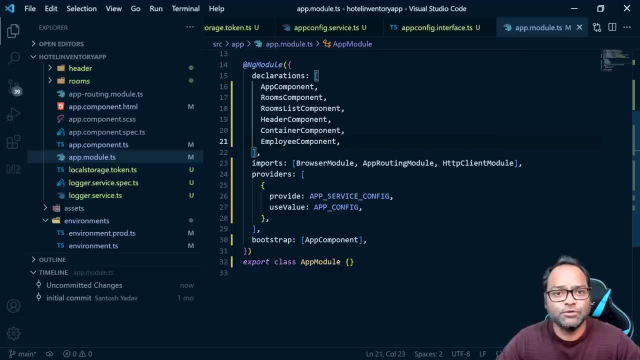 client module. as soon as you see module, it means this is something which needs to be registered at your module level. http client module generally should be registered at your root level because, uh, you are going to use http calls across your application, right? so you just need to register. 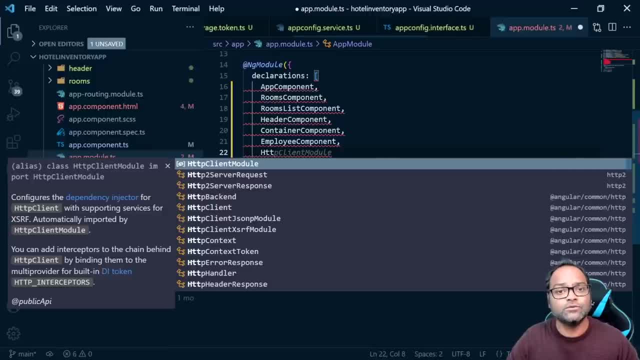 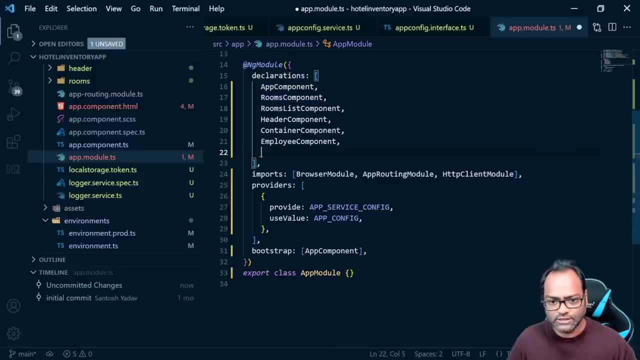 it once, and that's absolutely fine until unless you are using services, and even in that case this will be taken care of. okay, sorry, i just added it to declarations. really sorry for that. i okay, so here it is. so we have a cdp client module registered and we are going to use it as a 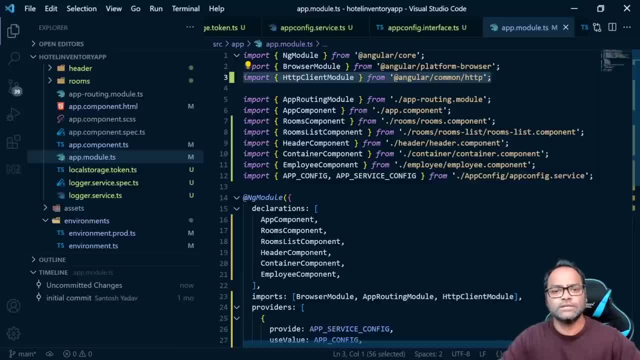 cdp client and we have imported it from angular common sdp. remember this angular common sdp because http client module should be imported from here in case you get an old code base. it's possible that, uh, there was another. uh, uh, there was another library called angular slash sdp. 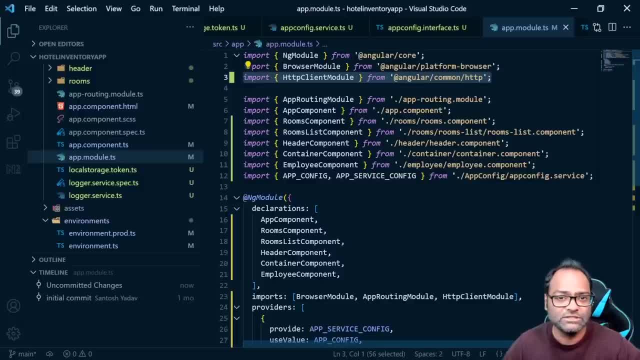 so if you are getting something from angular sdp, you are probably on the older version and you should move to angular common sdp, which was, of course, uh introduced in 2017, so you don't have to go ahead and still use that particular api. remember angular slash, common slash sdp? this is 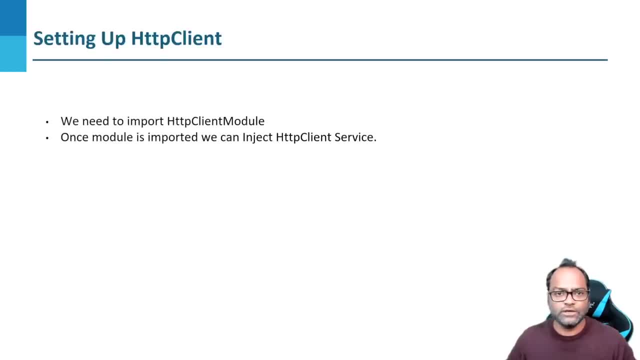 from where you should be using it. so this is first step. now we are done. we are done with setting up the sdp client. now let's go ahead and see how we can use sdp client service. but before we move into, uh, start using our sdp client service. we need an api and we don't have. 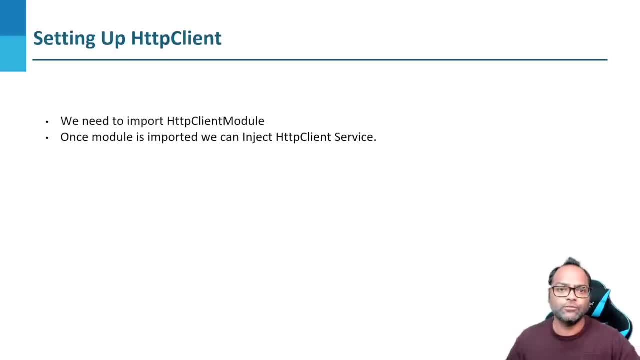 any api available as of now. so what we are going to do is we are going to use a mock api which i have created. you don't have to worry about this. i'll share the, we will share the code and you can just download it. this api is actually written in nest js. 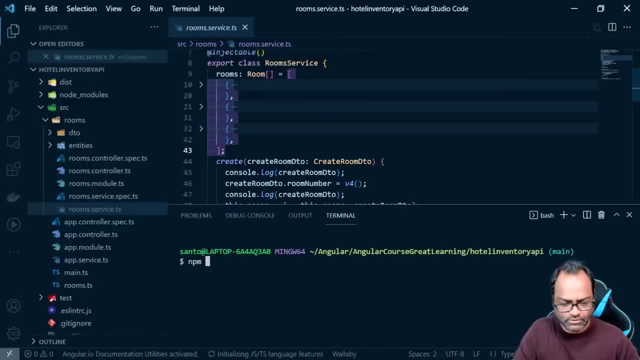 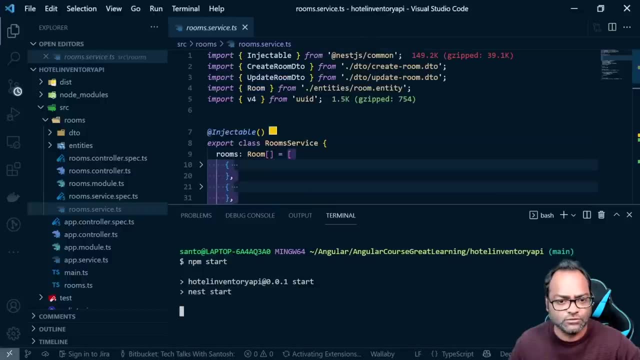 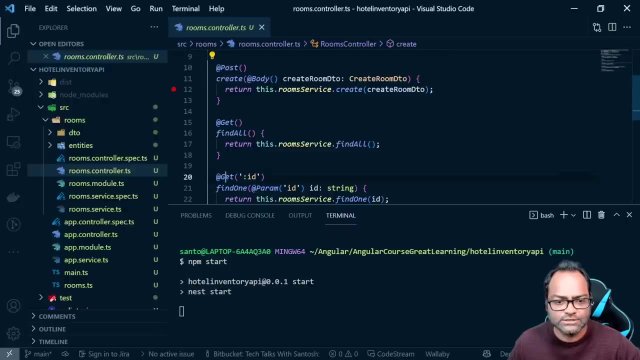 and it is written using typescript. so i'll just do npm, start here to start this particular api and it will expose some api endpoints which which we have already written, so you can go to rooms controller and you will be able to see api slash rooms. this is post, this is get, this is get by id and this is patch and delete. these are different apis. 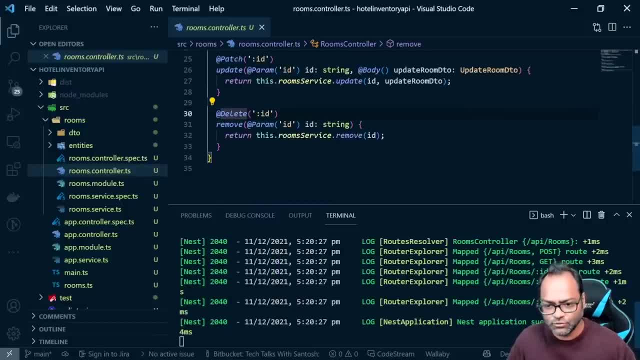 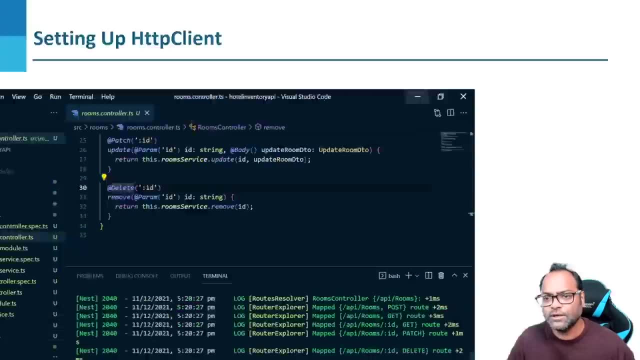 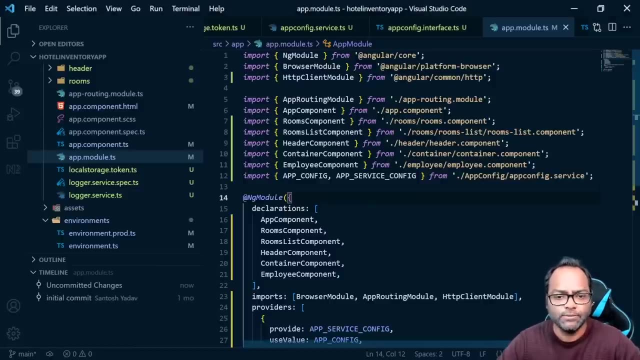 which is available and we will be interacting with this api. so you can see, these are the endpoints which we get: api slash rooms post. api slash rooms get. and now let's go back to our code base. uh, sorry, your uh. let's go back to our uh application. right, and the first thing which we need in case. 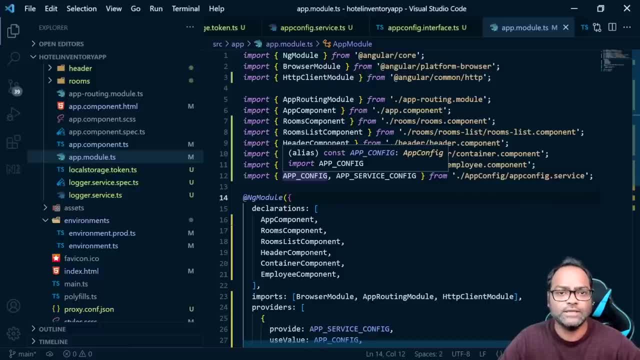 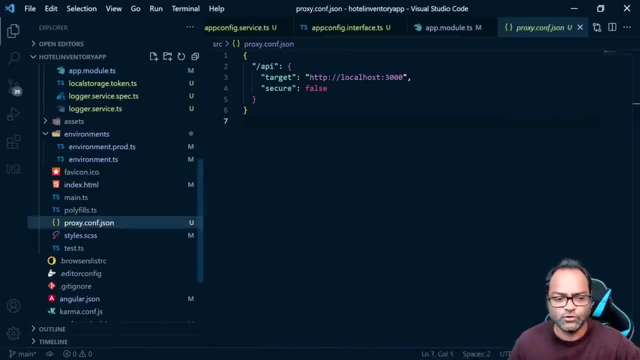 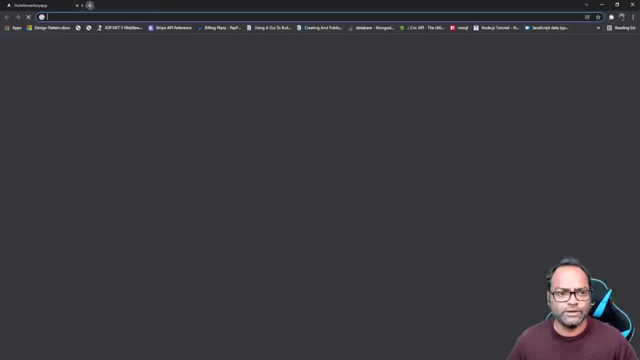 you are setting up your http uh or http api or your api server locally, you need to create one file, which is known as proxyconfjson. this is something, uh, there's something which is available inside documentation, so i'll just guide you to the document documentation and, in next time, whenever you want. 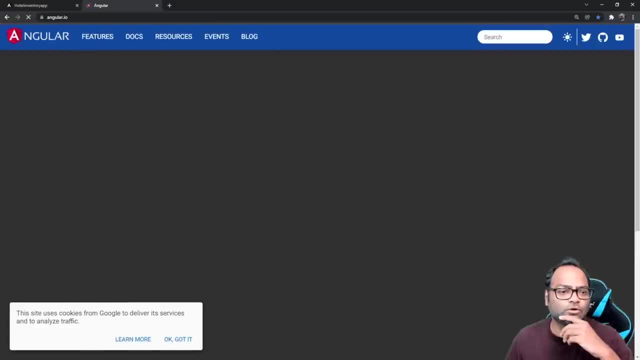 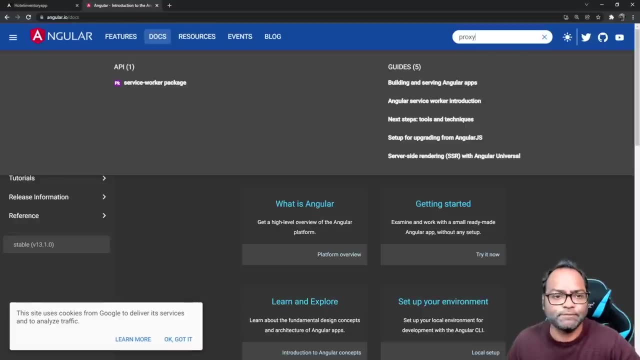 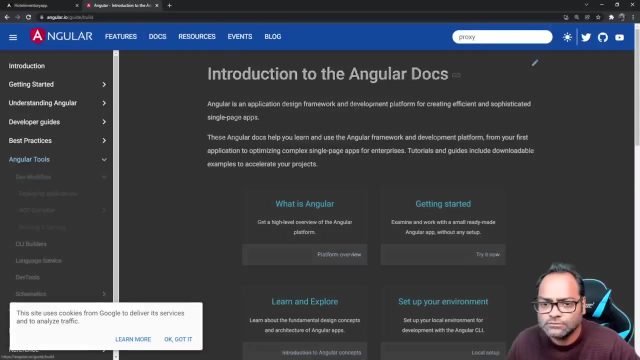 to set it. you can just refer the documentation. so you can go to angulario, which is, of course, the official documentation, search for proxy and you can search for proxyconf and now you can see your api asks me to open up my api. so this will help your api server because when i go to proxyconf i'll have a link to that. 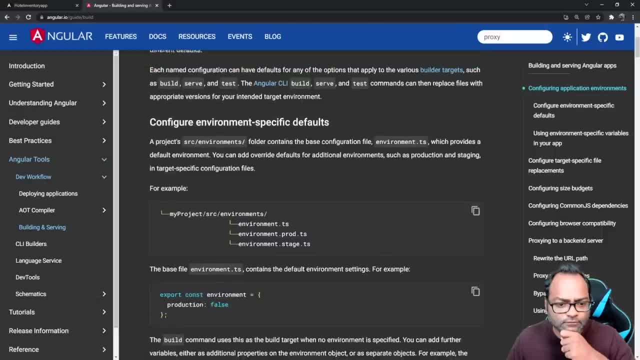 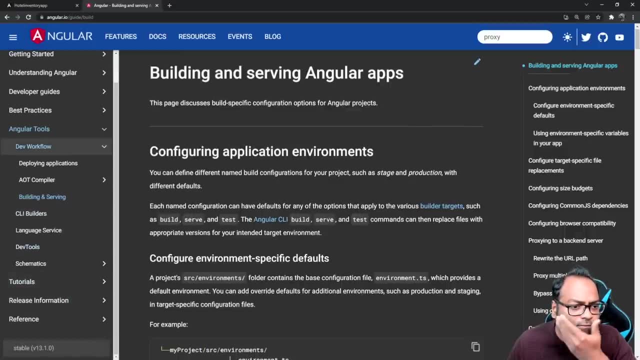 so i'll select proxyconf and i'll see what i have here. there's a post here where i'm going to create a private api. i'm going to select proxyconf and i'm going to click on proxyconf and it'll prompt me to take a test. so we'll just go up to proxyconf and i'm going. 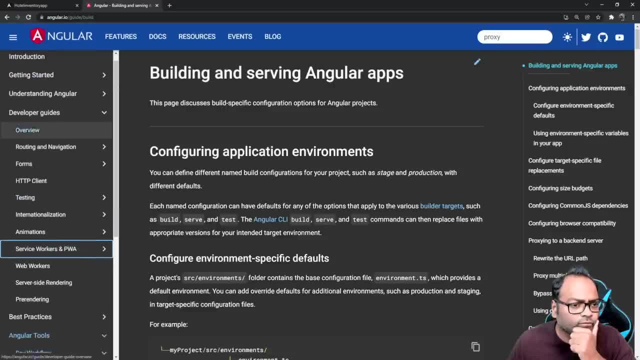 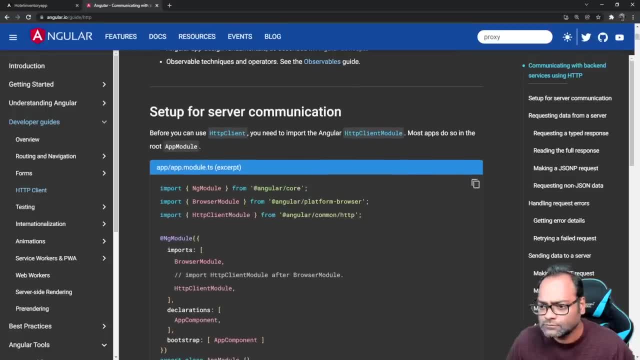 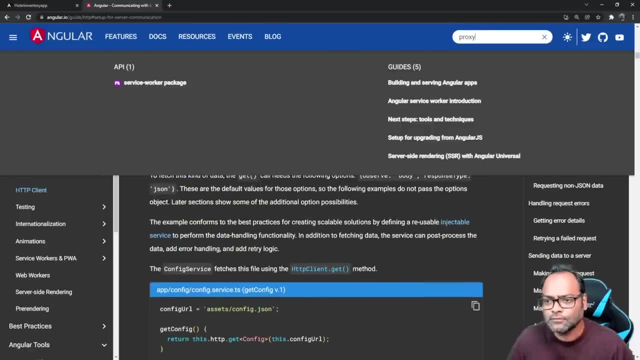 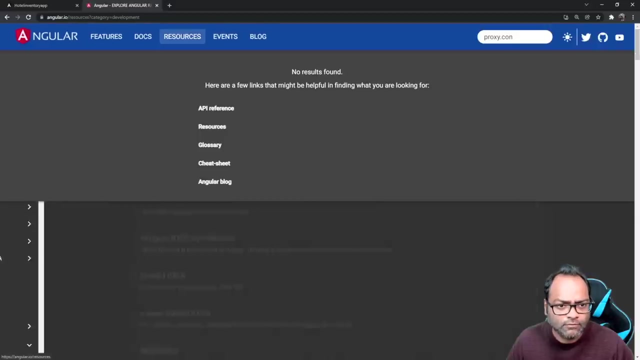 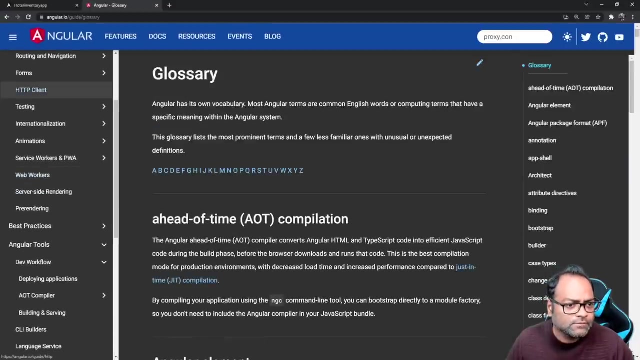 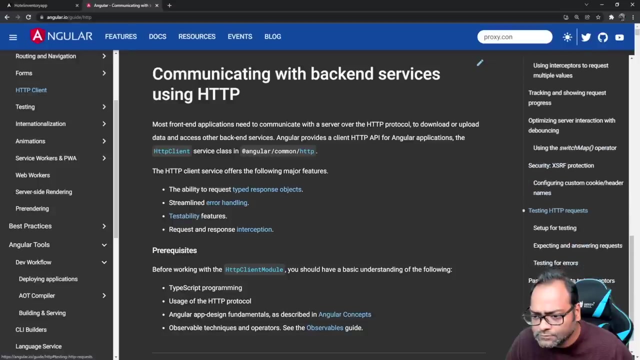 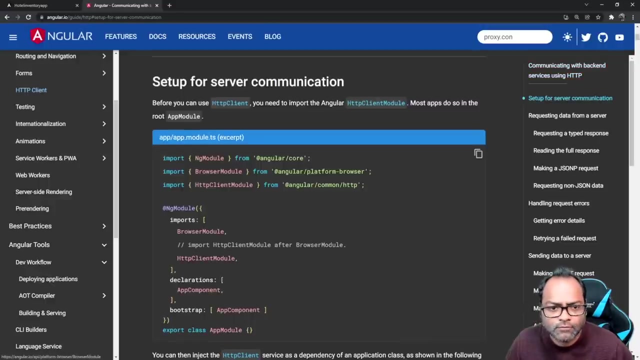 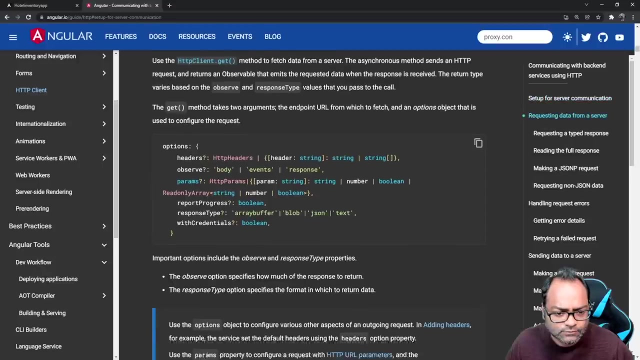 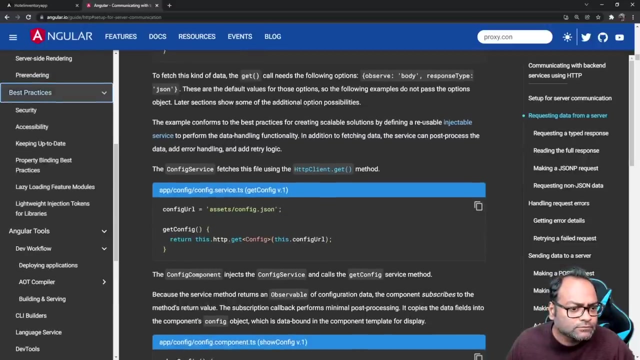 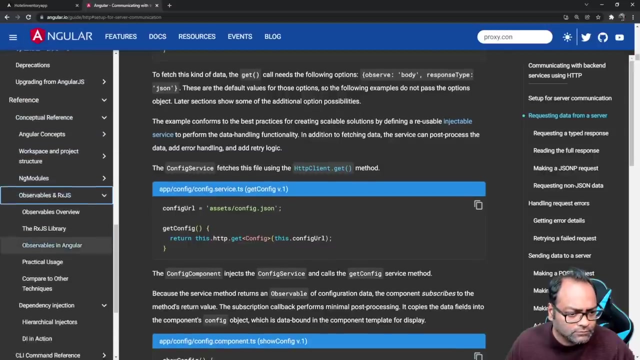 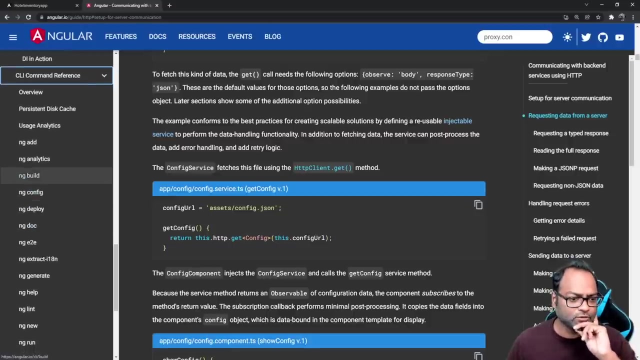 to make sure it's pretty consistent and i'm going to say a normal code and i'm going to: Mm-hmm. Okay, let me see, Let me get this set up, okay here, Mm-hmm. So yeah, you can go to the documentation and go to this ng-serve command. 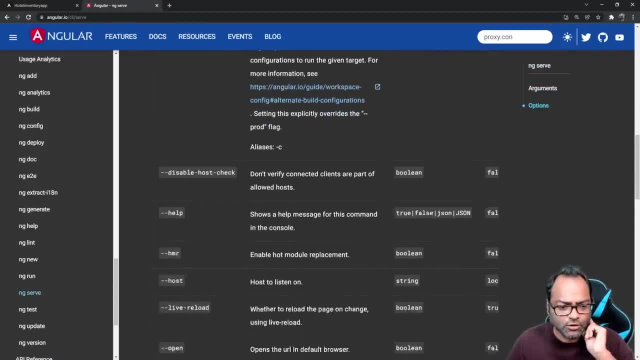 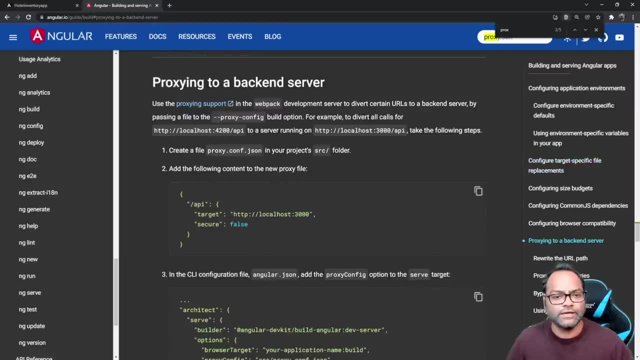 And in ng-serve you will find one property called proxy, Proxy, Yeah, Proxy config, And you can just click here. It will take you to the page where all the information is available, So we can create a proxyconvjson. 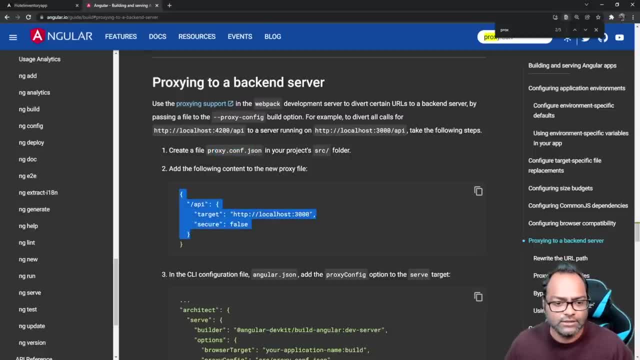 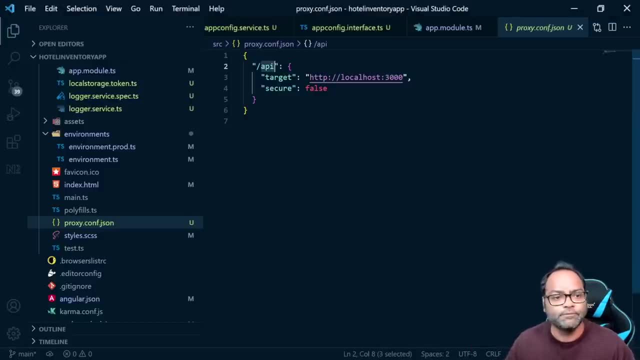 This is first step, which I have already done for us, And then you can just copy and paste this. Our API also exists with slash API, right? So slash API slash, Sorry, slash API, slash room. So we'll start with slash API. 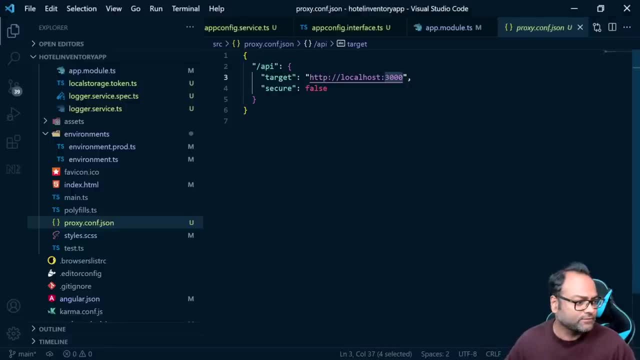 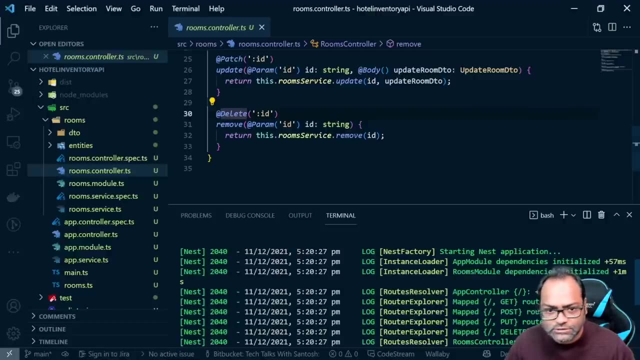 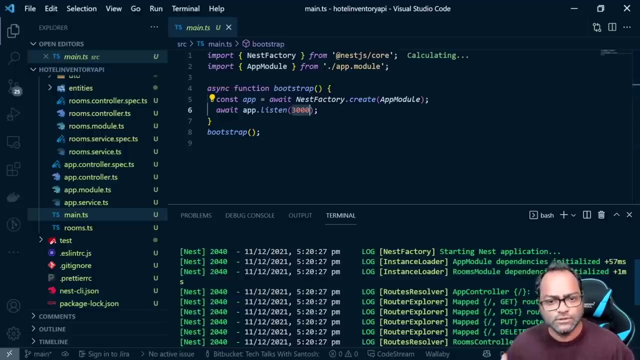 And this is where the API exists. Okay, So we'll start with localhost 3000.. So you can verify from here this application maints and applisten. So right now it is running on localhost 3000.. And after this there are a few steps more, which I have already done for us. 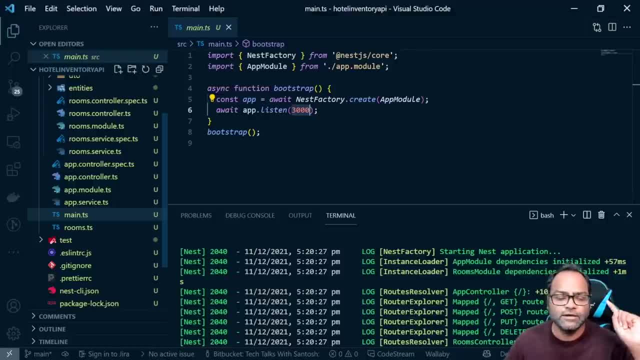 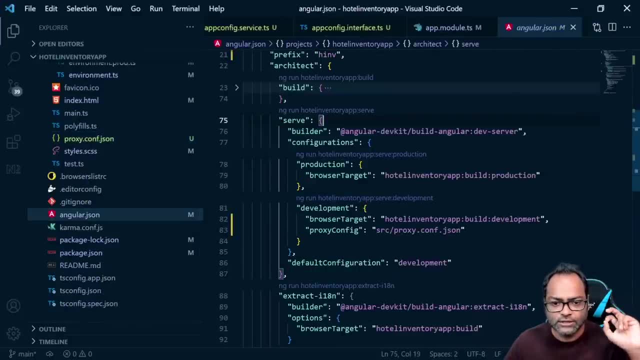 But you can refer it from here. We have to actually add one more configuration. So we have to add one more configuration inside our angularjson: The serve command. This is the configuration for serve And we have added this inside development. We have also added proxy config and path to our proxyconvjson file. 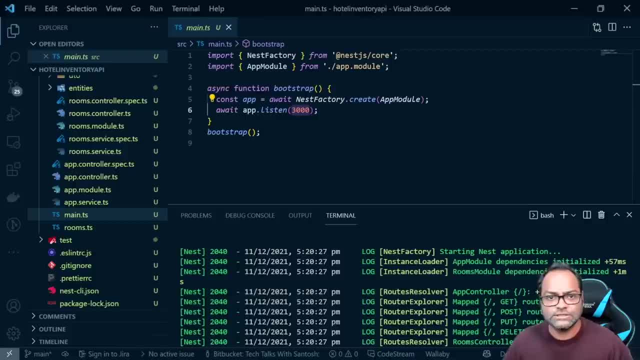 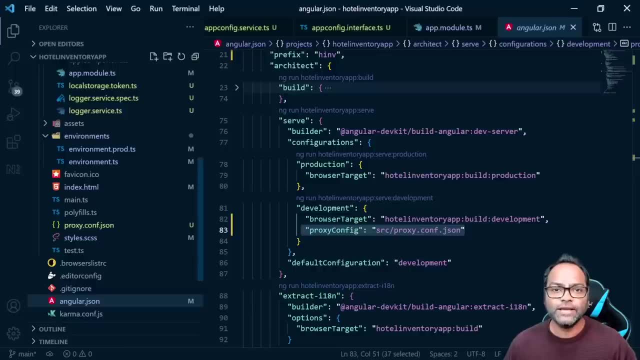 Once you do this, that's it. You're done, Right? So this is to set up the proxy, And now let's go ahead and utilize the service- http client service- to make our first API call. So, room service. 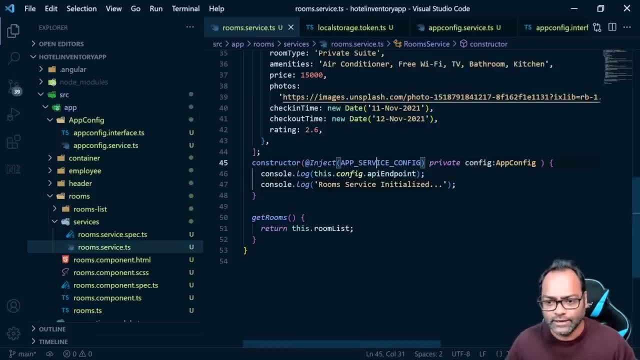 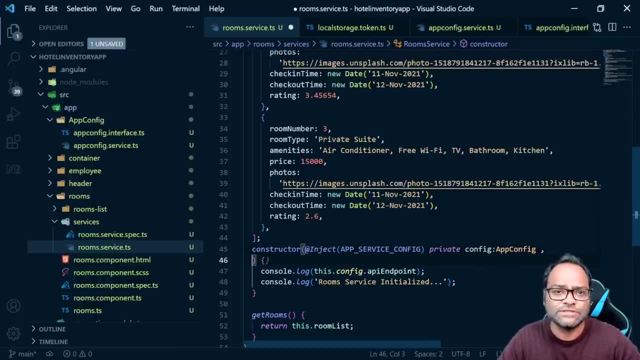 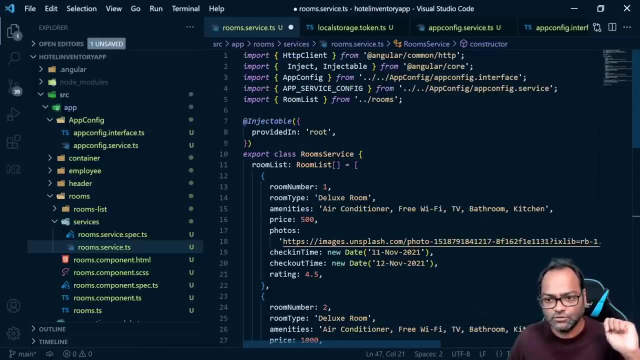 This is where we want to go And we are going to use http client service, which is available inside Angular. So we'll say private http And we'll say type of http client. Let me just remove this And we will import http client from angular slash, common slash, http. 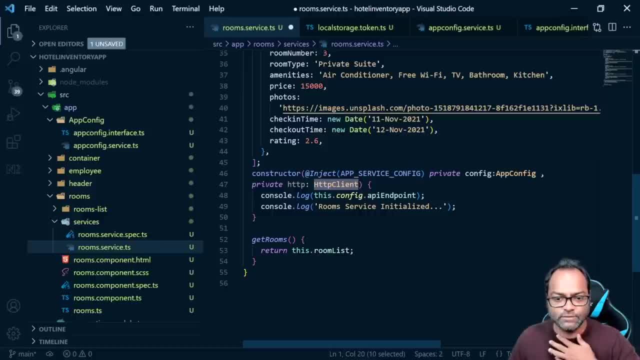 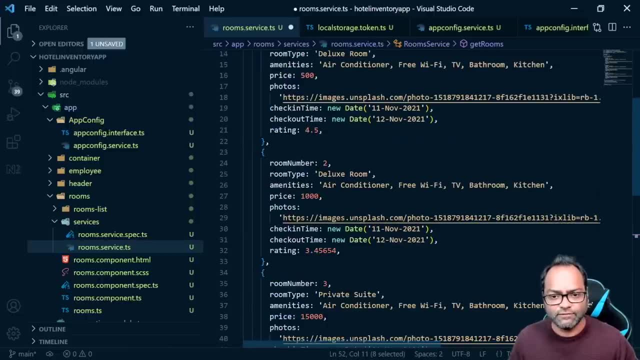 So this is imported. Now we have our http client service available, Let's go ahead and make our first API call. So here Now we are getting the data from, of course, service itself. We have encoded this data. 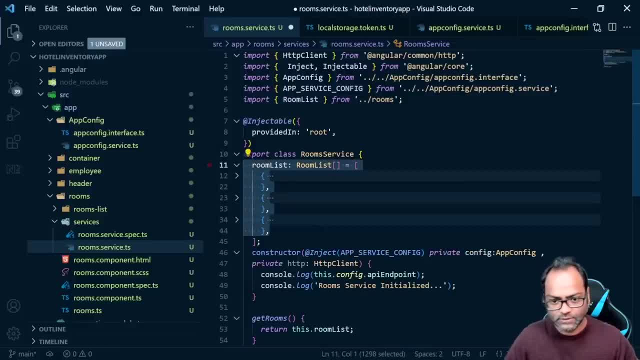 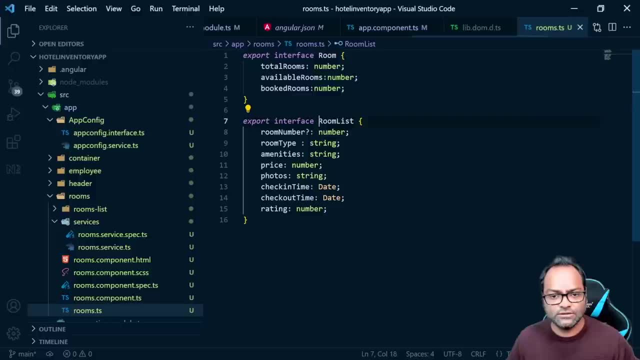 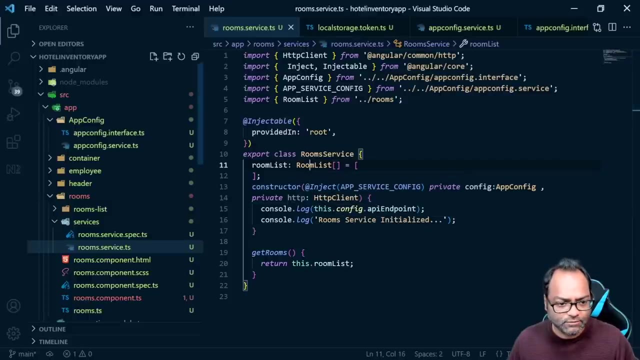 Let's remove this. Let's get rid of it. I'll do one small change: As my ID at the back end is a string, I'll change this room number to be string And probably I have to change at one more place, which is this: 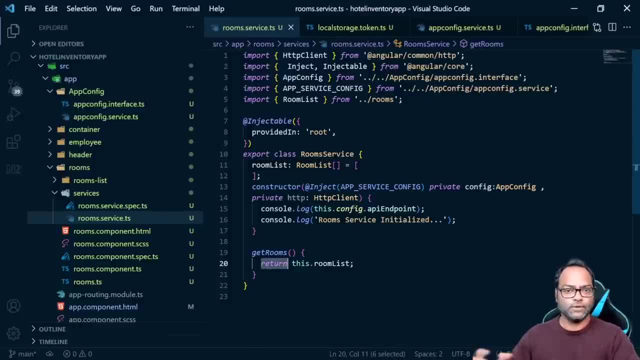 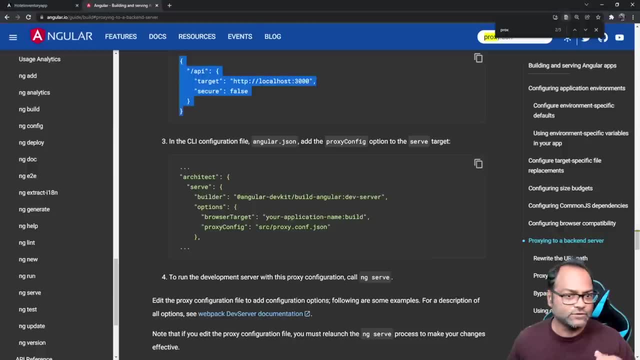 Now to get the data from an API. we generally make a get call, So get calls can be accessed from the browser itself. So let's try to see if that works. So I can say: localhost 3000, slash API, slash rooms. 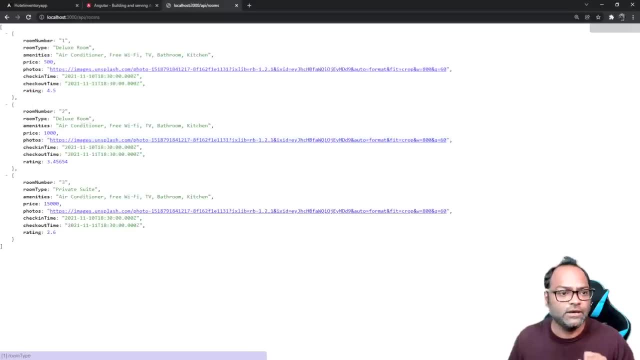 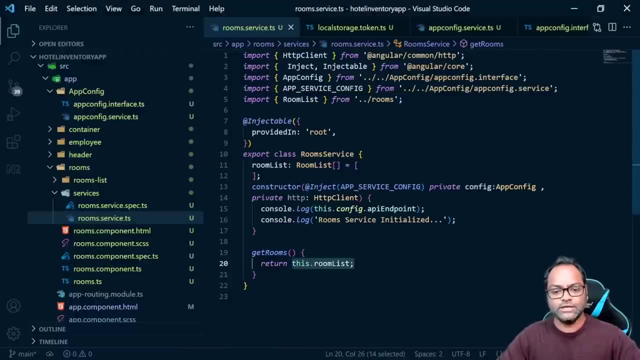 This is where our resources are available, And you can see we have three records available already And this is our data. So here, rather than actually getting the data from this dot room list, what we are going to do is we are going to call the HTTP get method. 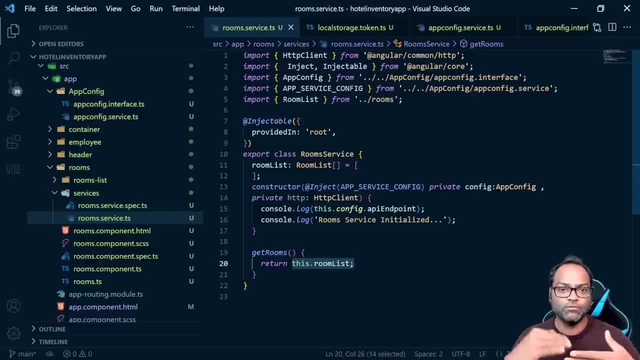 So there are multiple methods which exist. So we have get post put, delete patch, And there are a few more, but we won't be using them a lot, So let's use Generally. we call like whenever you start working with a new framework. 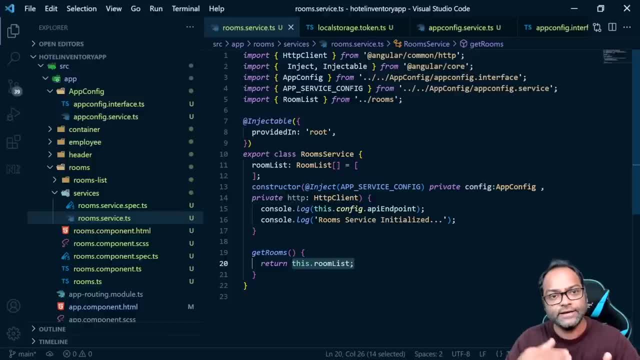 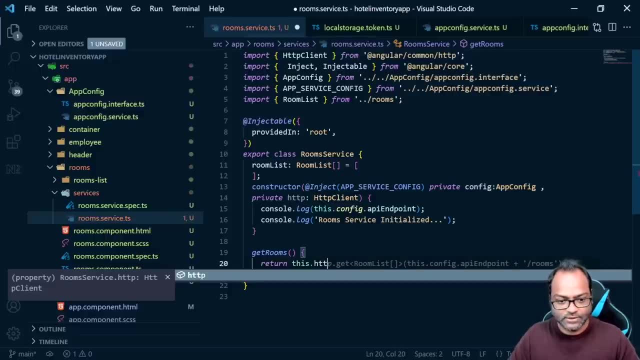 the first thing which you learn is CRUD operation: right, Create, read, update, delete. That's what we are going to do. Get method is read, So here I'll say this: dot HTTP, dot get, And you can see I'm getting intelligence, but I'm not going to use it right now. 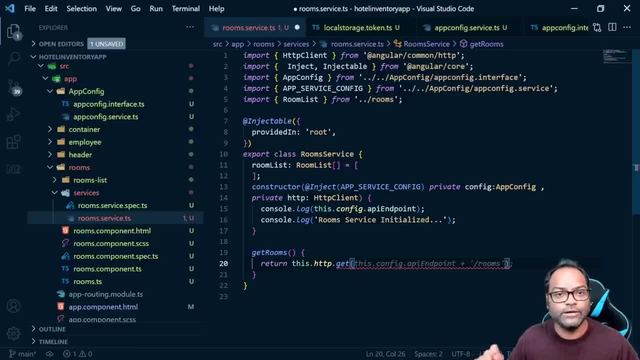 So I'll say: HTTP get And we need an API endpoint Right now, as we have a proxy server available, we don't have to give entire path, So we don't have to mention localhost 3000, slash API, slash rooms. 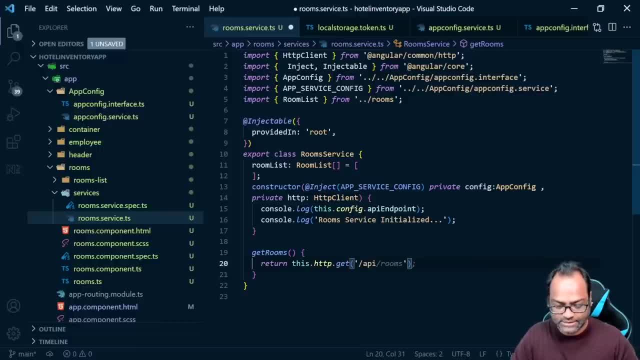 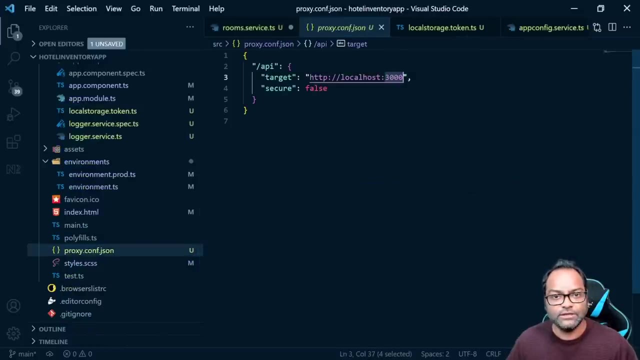 What we can do is we can mention slash API slash rooms. This is it because of the proxy config which we have. So proxy will redirect our this call slash API slash rooms to localhost 3000, which is available here Right. And now let's say: let's save this. 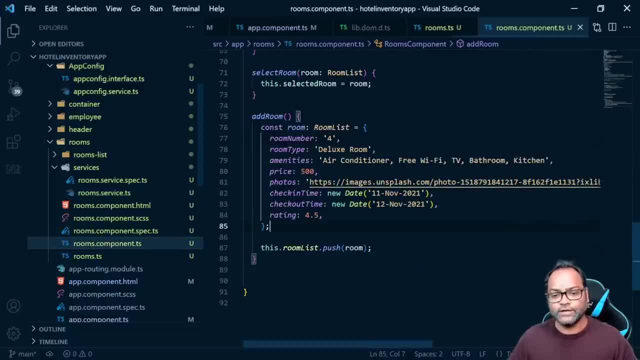 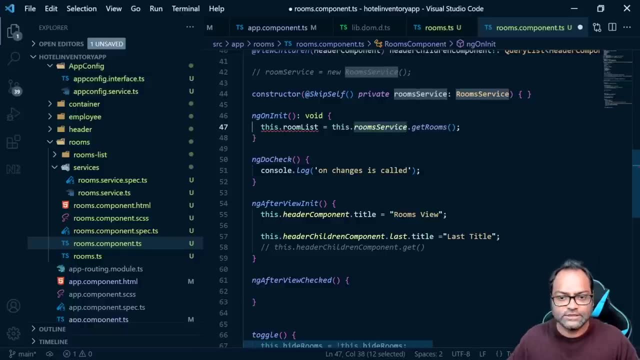 And once we go back to our component we will start getting an error here. So this code is commented right now, but let's uncomment And we will start seeing an error. It says this dot rooms has some swiggly lines. 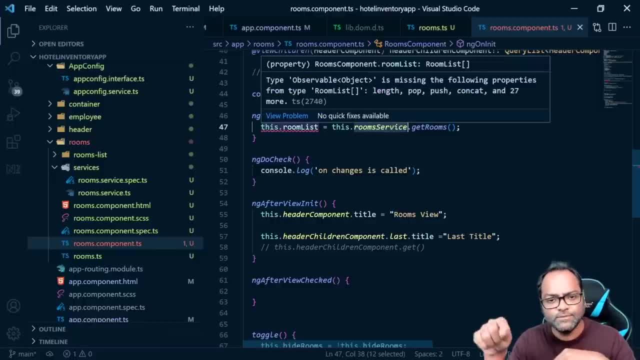 Let's see what it says. It says type: observable of object is missing following properties. So it is saying: okay, whatever data you are trying to actually assign this, assign it to room list- is of something of type called observable. What is this observable? 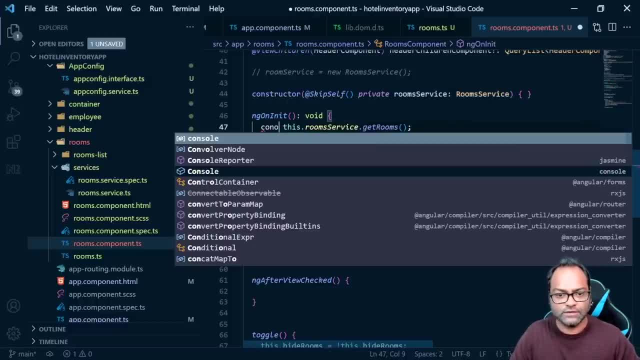 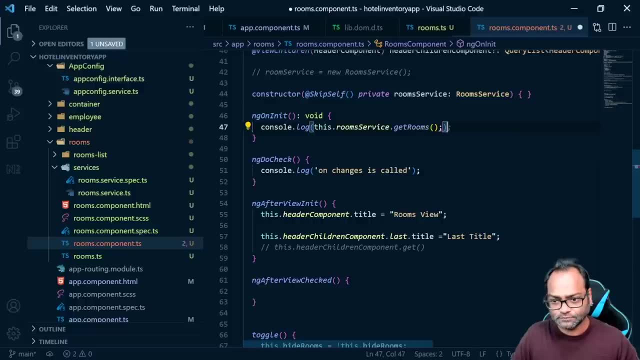 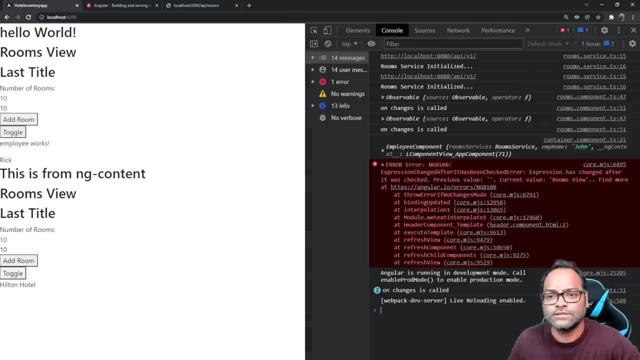 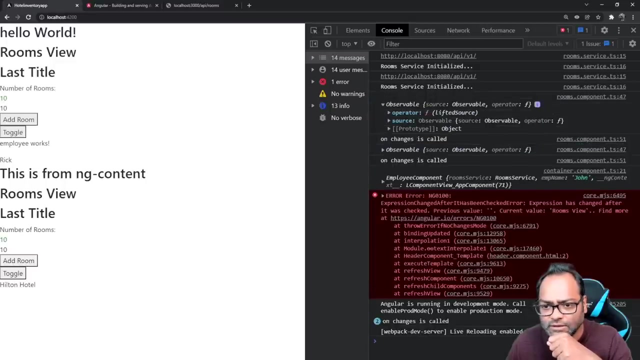 So let's see this first. What I will do is we'll just do a console dot log to try to understand what this observables and everything is, And let's go to the console And we can see this Right. So we have observable which says operator, and there are something called source. 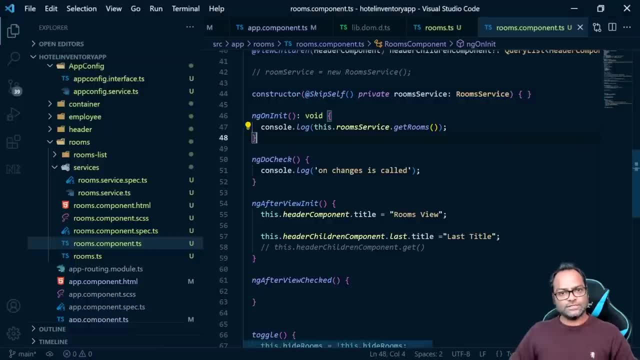 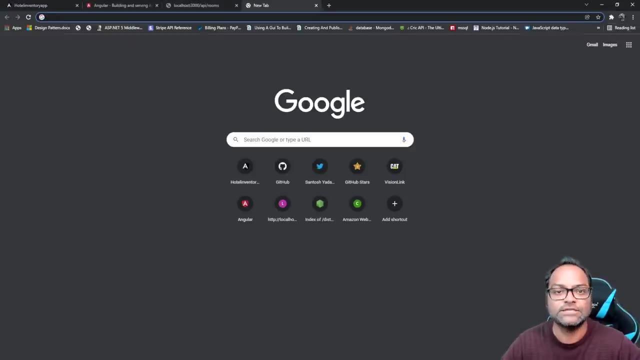 But there is no data, So let's try to understand what observable means. Angular uses a library called RSJS internally to work with data, And it is also used inside your HTTP service as well. Even there are a few other places like. we will be using it in forms. 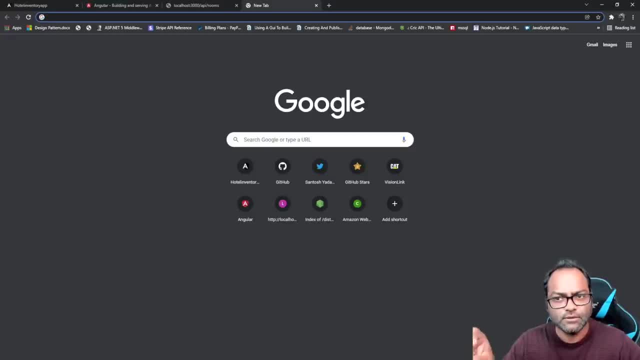 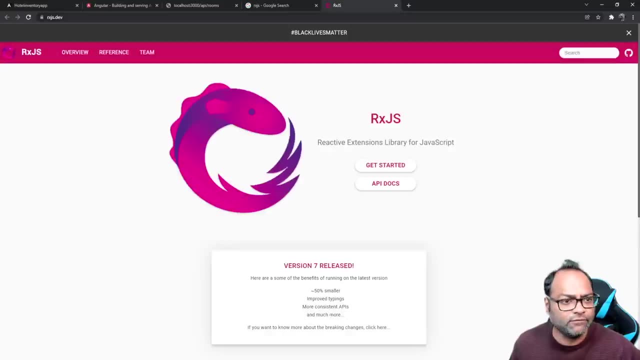 We will be using it in routing. So multiple places, So RSJS. let's see what is this. So this is the official web page here: rsjsdev, So you can go ahead and see what RSJS is. 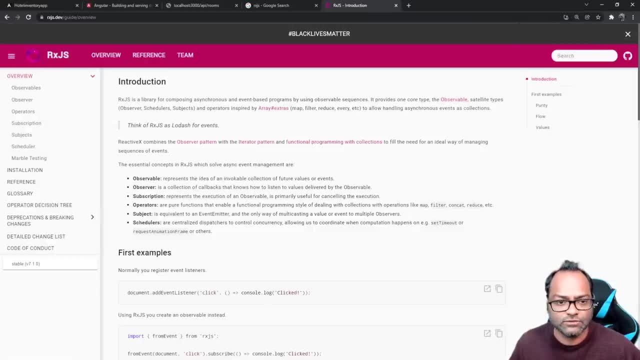 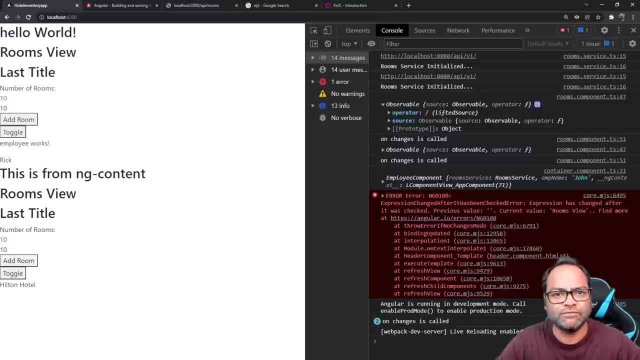 So there is a small introduction which is written here. So it's a library. It's, of course, a library to work with event-based programs using observable sequence. So what do you mean by observable sequence? I mean, probably you might have never heard about observables. 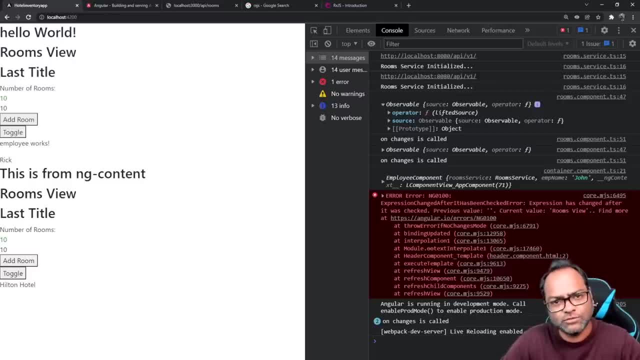 Because it's of course a different library and generally we don't use those libraries. But RSJS is one of the powerful libraries which is available here And can be used with any framework. So it is not that it's only technically coupled with Angular. 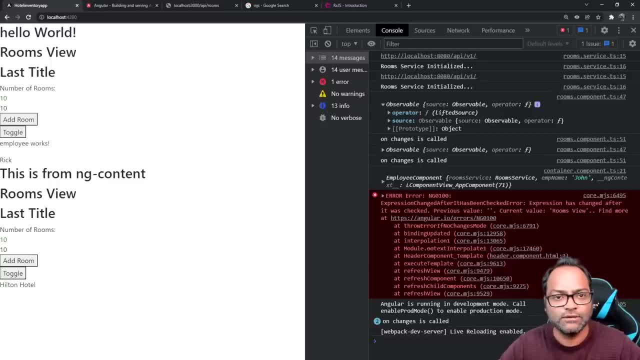 It's used in React, It can be used in Vue, It can be used in Svelte, Anywhere you want. So RSJS has a concept that whatever data you get is a stream of data, Right? So what do you mean by stream? 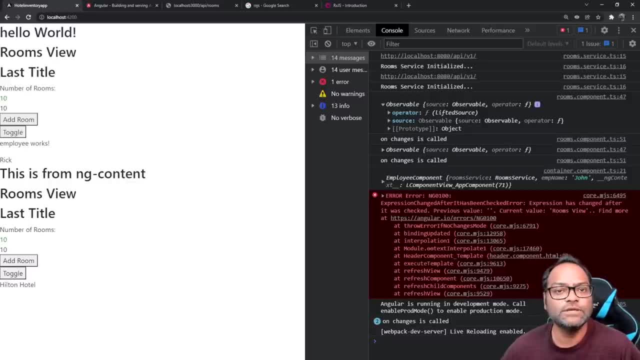 For example, you might have already used a lot of streaming services. So let's go to YouTube, Let's go to Netflix, Let's go to Amazon. What are those? They are your streaming services, Like Amazon, of course. Amazon, not the shopping app. 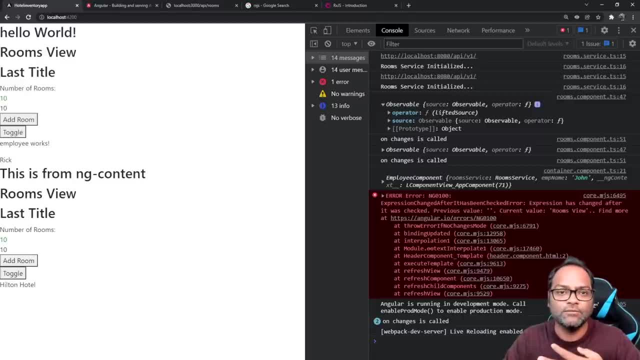 Right, Amazon Prime. So what you get is you get stream of data, Right? I mean they are streaming some data to your devices. Once we say stream, So it's like once you, What happens when you want to access some streaming services? 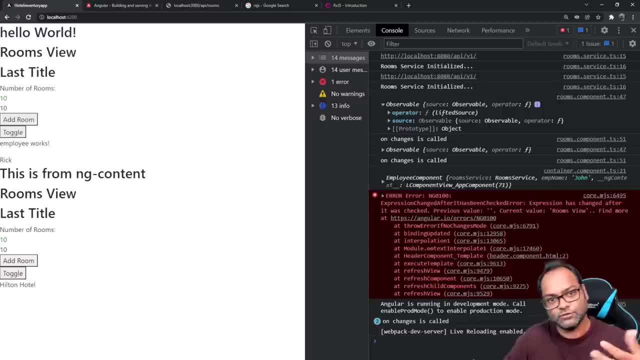 The first step is you subscribe to it, Right? I mean, of course, you need to create an account, You subscribe And then you can start getting those streams. The similar concept works inside RSJS. So once you want to get some data, the first thing which you have to do is you have to. 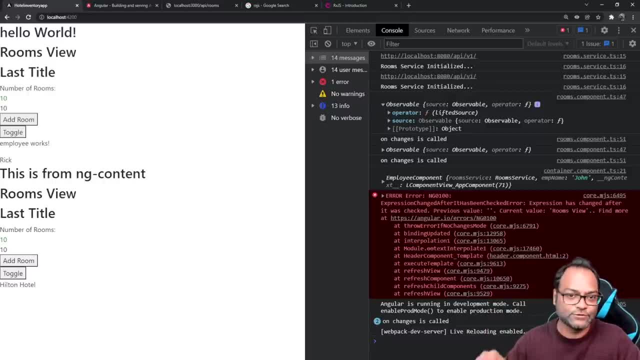 of course, someone needs to publish the data. That's, of course, true, Because, of course, if no one is publishing the data or no one is publishing the streams, you will not get anything. But as a user, as a developer, what you should be doing is you should be subscribing to the 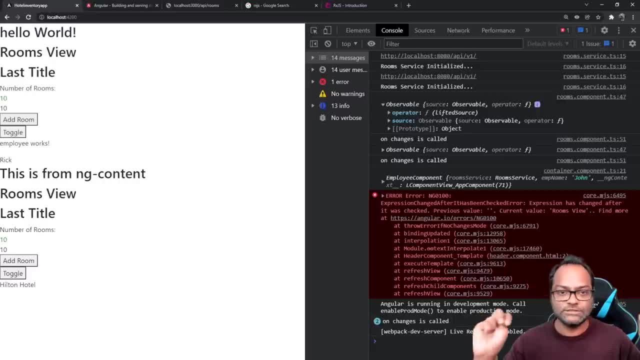 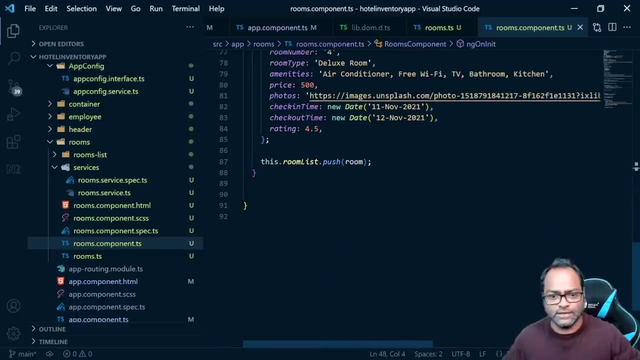 stream to get the data. It's a continuous stream Generally. let me just try to explain you a common term which is used a lot, called push versus pull architecture. Let's go back to our code base. I'm not going to write entire code, but yeah, just an example. 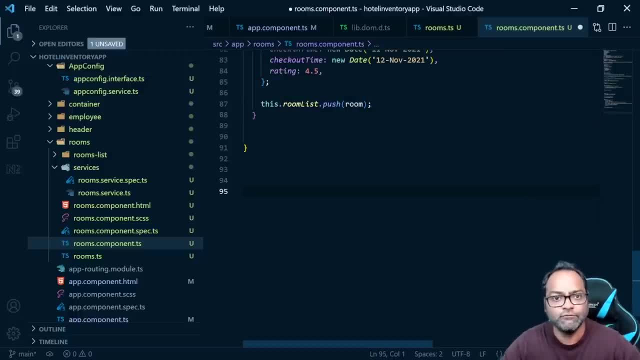 So here, Let's say, if we are not using stream, what you will do is you will call, let's say, get data, to get the data. In case, let's say, we perform some operation, We add the data. So we add a new data. 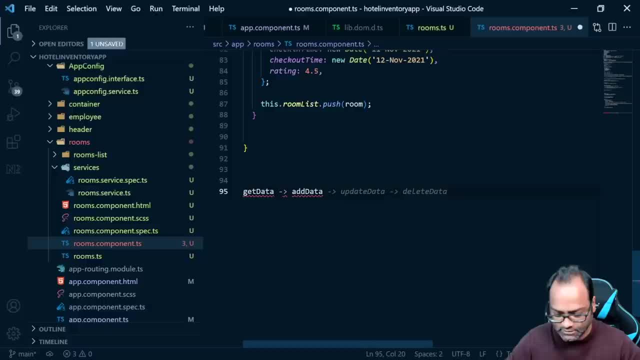 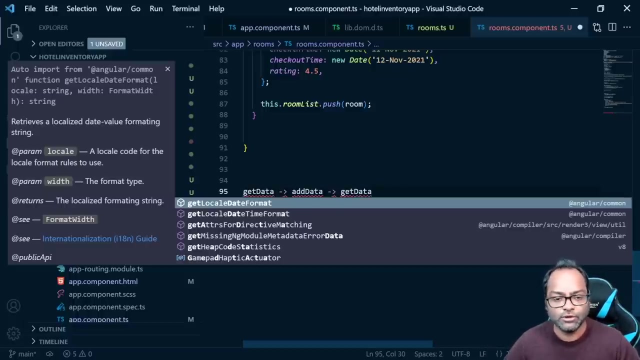 What you need to do is, in case I want to get the latest data generally we do- is call the get data again. This is something which we have been doing from a long time In JavaScript. we have been doing from a long time. 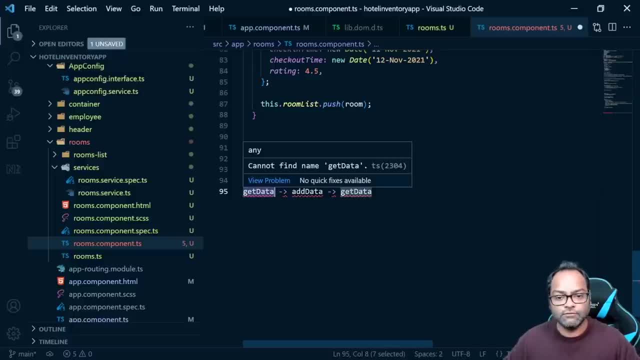 So whenever you modify the data, what you do is you get the data again. What you do is you pull the data. This is called pull-based architecture. So every time you update something, just go ahead and pull the data. RxJS works on a push architecture. 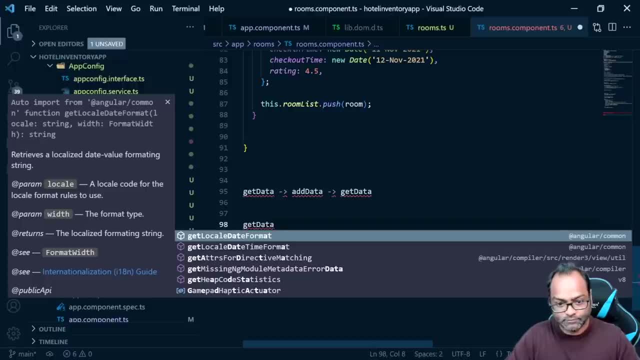 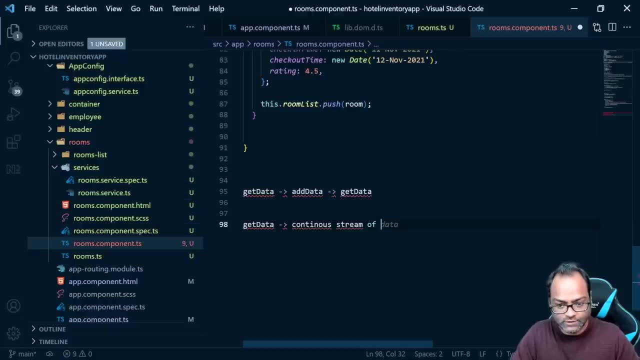 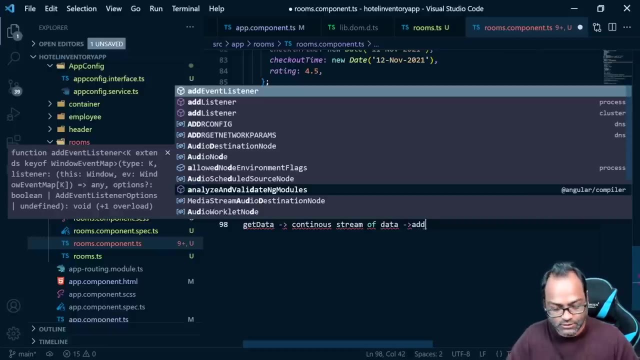 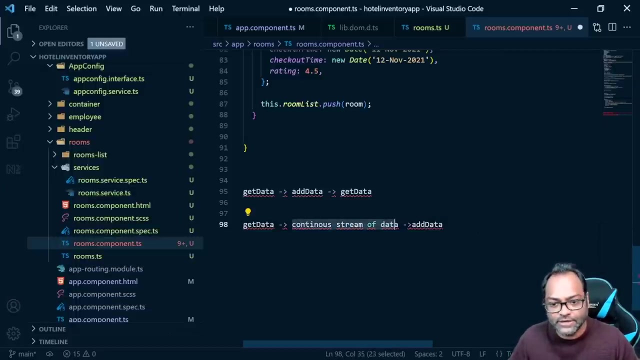 It says: once you get the data, it is continuous stream, Continuous stream of data. So, in case you add some data, you add the data directly into the stream And once this stream is updated, anyone who has actually subscribed to the stream will. 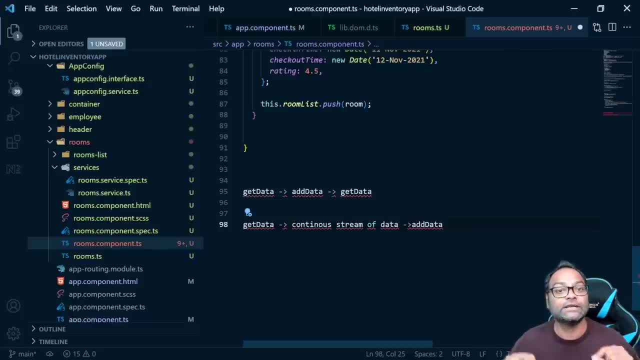 get the data. You don't have to call the get data function again To get the data. That's pull-based architecture. Here we are saying: whenever you update the stream, you will get the updated data. That's push-based architecture. 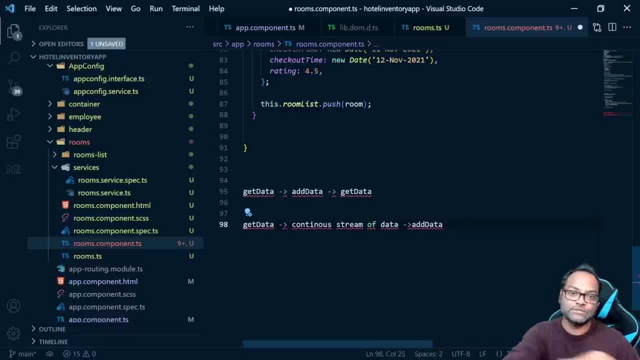 You are not doing it yourself. Actually, stream is pushing the latest data to you, So hope you understood this, because this is really important to understand RxJS and streams. I'll just leave it here in case you want to refer this again. 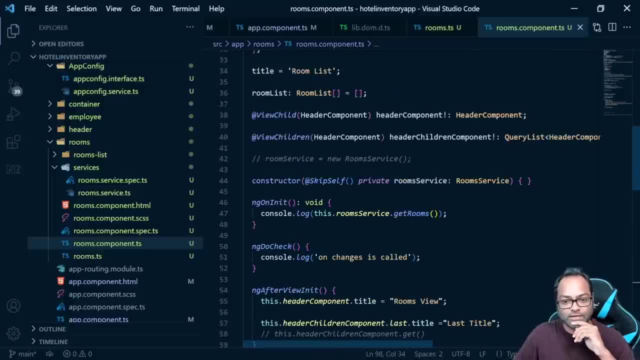 So what we are going to do is we are going to get our, of course, stream Rooms data First thing. in case. I want to access this data, what I have to do is I have to go ahead and subscribe to it. 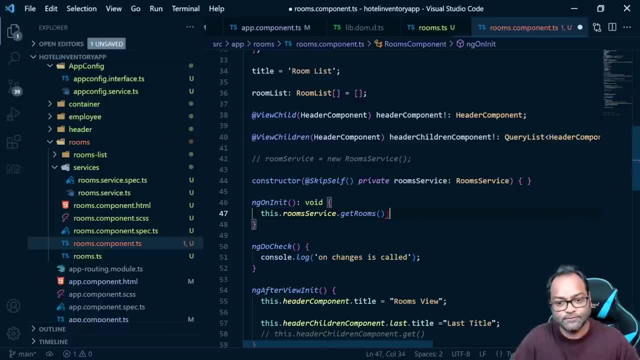 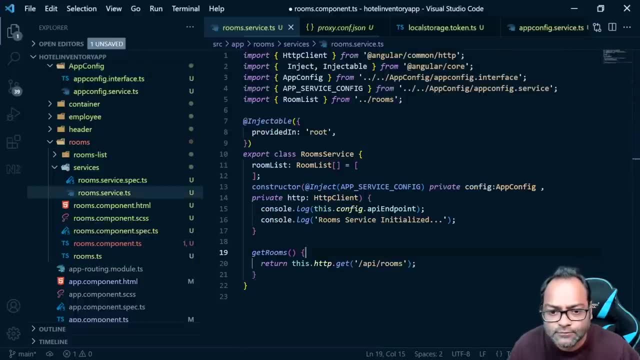 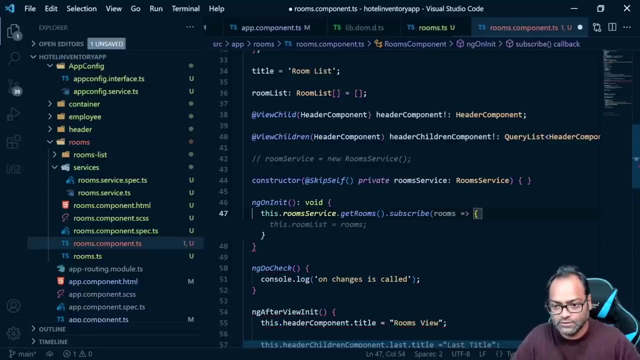 And how we can subscribe using RxJS. It has a subscribe method. So you can do: get rooms, dot, let's see subscribe, And here we can say this dot, rooms list is equals to rooms. But we are getting an error. 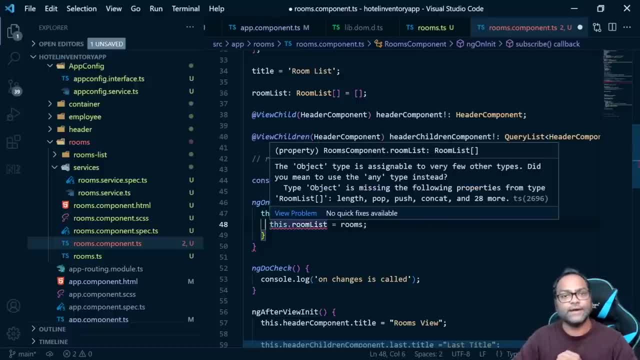 Again. I mean why. Let's try to read the error. This is one of the most important skill you should learn In all the modern or the latest frameworks which we have available nowadays. the developer experience is really. developer experience is really great. 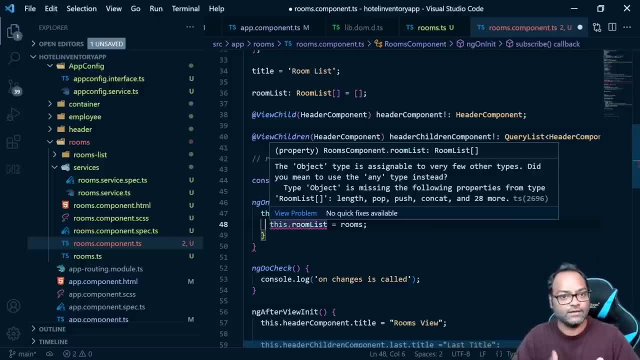 What do you mean by developer experience? So it's all these things right, Errors or messages while developing. So it guides you what the actual issue is. So it says that this room list is of type this room list array. 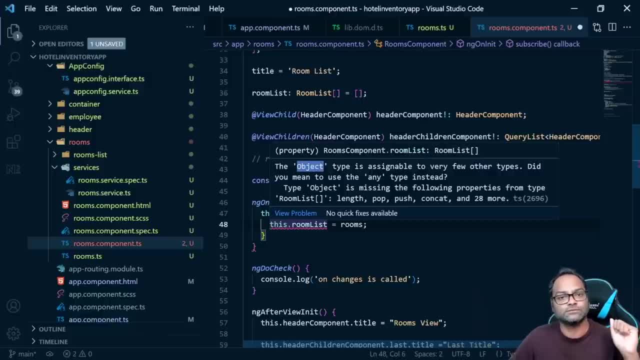 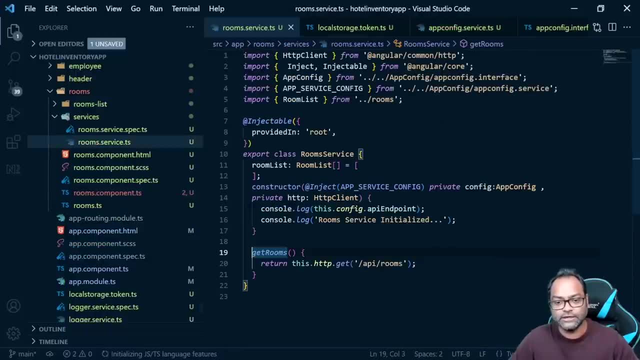 But you are trying to assign it to an object And of course there is a mismatch in data type. What we can do here is we can go ahead and change in get rooms. We can actually ask our HTTP service to actually give me the data in this particular type. 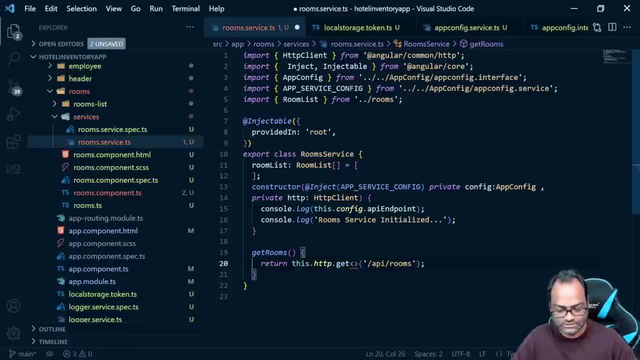 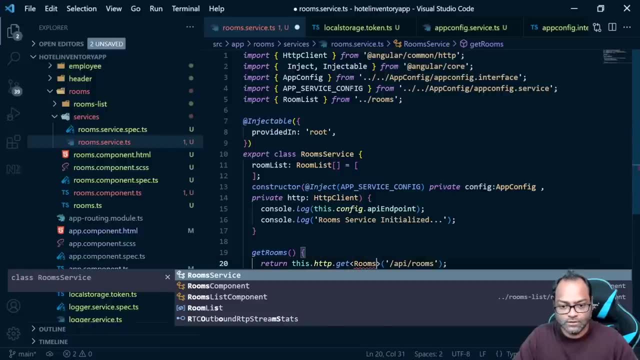 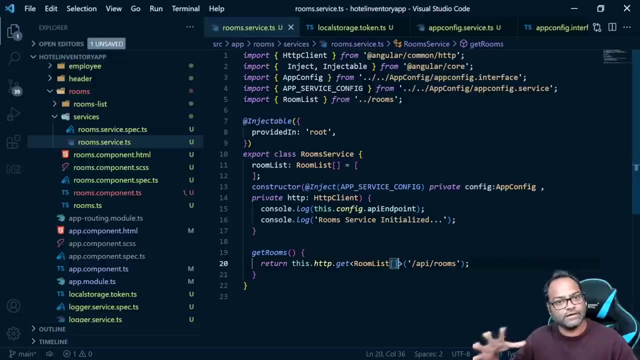 So I can use these generic syntax And I can say: room list, So room list array. So we are saying: whatever data I'm going to get, just transform the data into this particular object and then give it back to me. 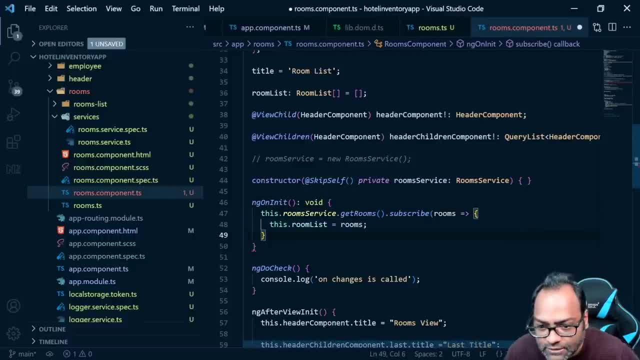 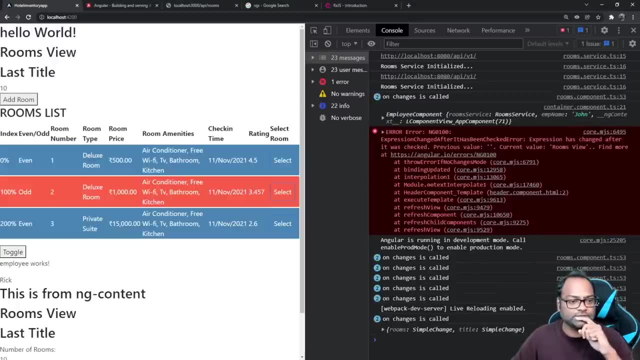 And you have your data available. And let's see what else we are missing. We are just missing one packet And let's save this. And let's go back to our front end And let's click on toggle And you have the data. 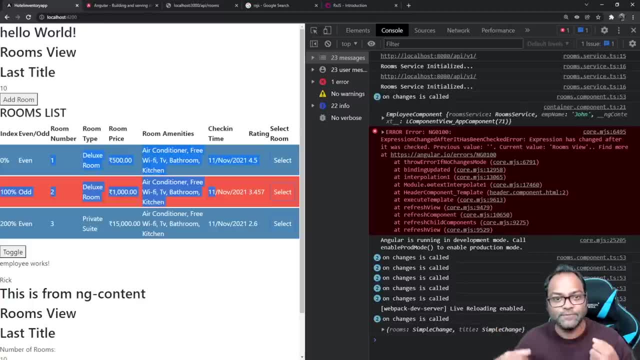 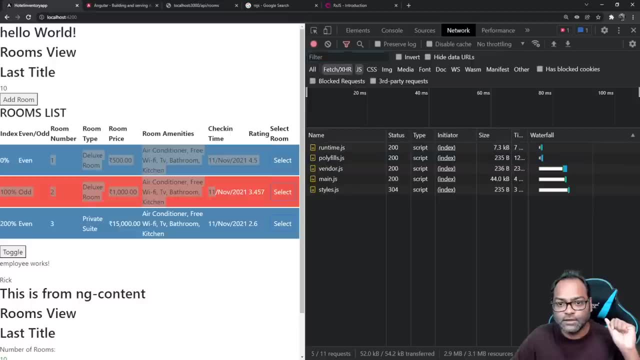 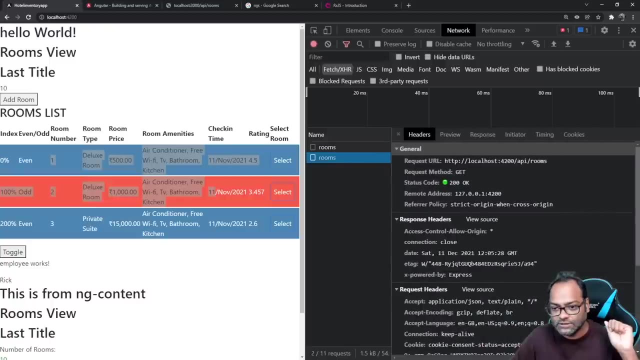 You just made your first HTTP get call from an API using Angular. You can go to network And you can just go to fetch XHR And you will be able to see your request. So here we have our get request, which returned us status code 200. 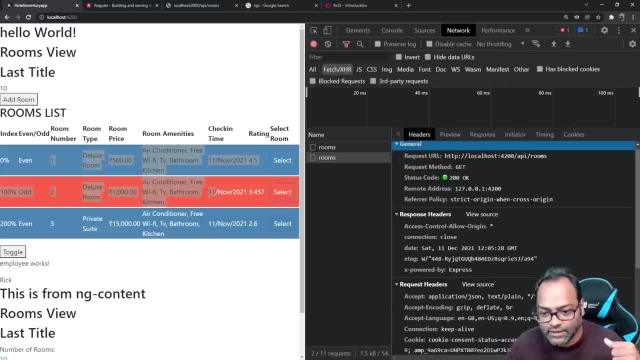 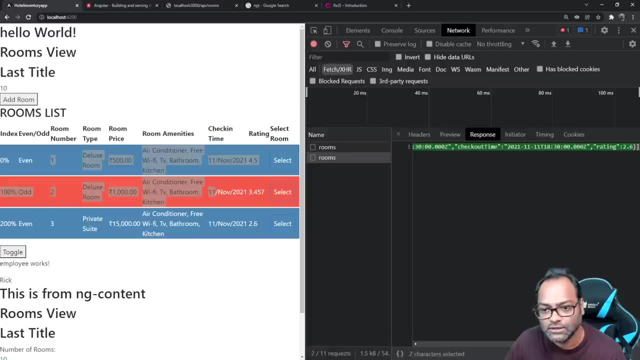 You can go to preview to see the data which is written, And these are request headers and request requests. So this is your plain JSON response And this is your formatted response, And it also tells you when it started and how much time it took. 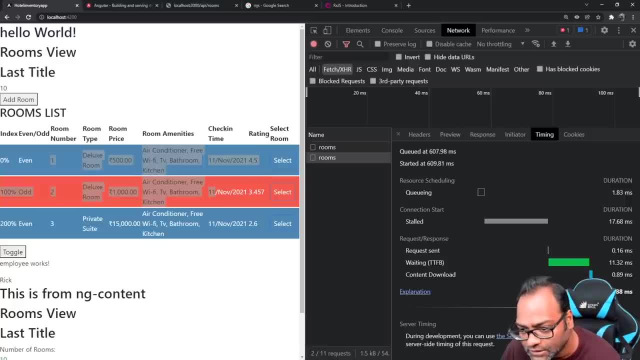 So it was completed around in 0.89 milliseconds. So this is how much it took to actually download the content. It was waiting for 11.32 milliseconds to complete the call, But total, if you see here, It's 31.88 milliseconds. 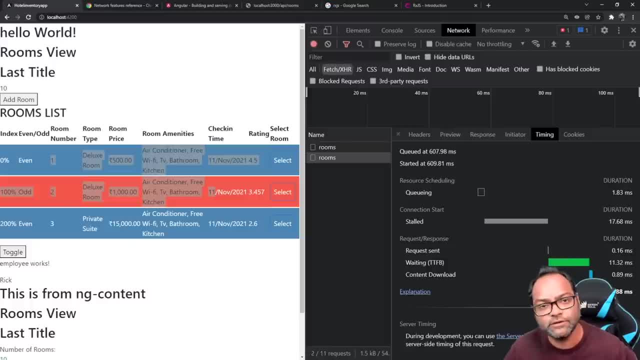 So this is absolutely fine. I mean you should not. Your API should respond within one second, And 31.88 milliseconds is perfect. I mean, of course, it's a local database And we Sorry, It's a local API. 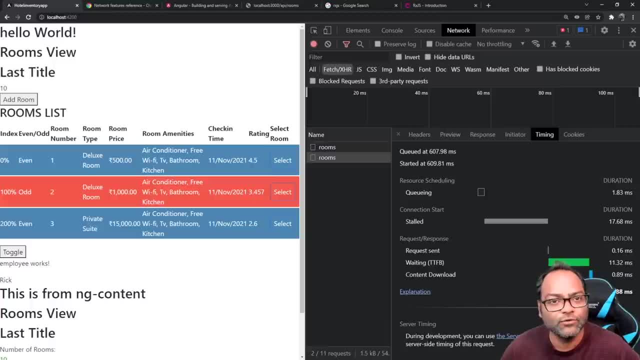 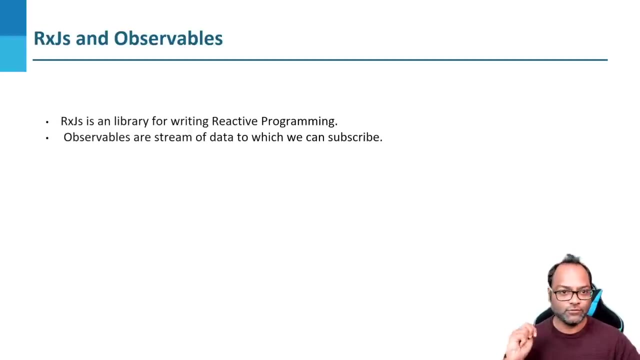 And we just have three records to fetch. But yeah, Congratulations, You just made your first API call And you have rendered the data on your UI, So now we understand how to get the data from HTTP, But I'll focus again on RxJS, because this is really important to understand. 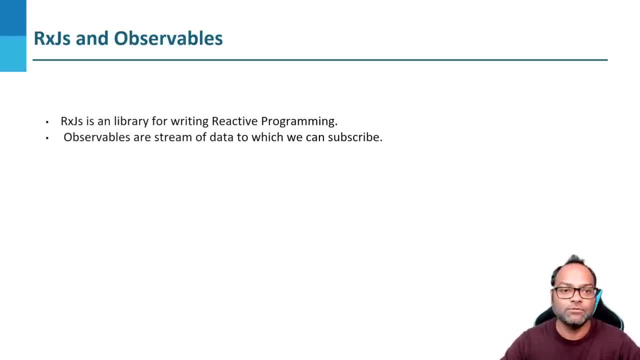 So we saw that, okay, RxJS is something which gives you a stream of data And it is used for writing reactive programming, And we also discussed about pull versus push. What is the difference? And it gives you like, it gives you observables, like stream of your data which we can subscribe to. 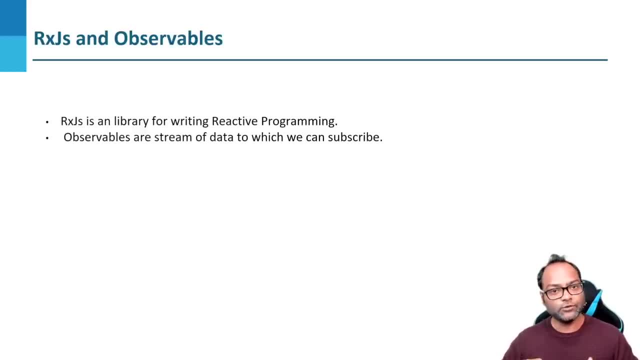 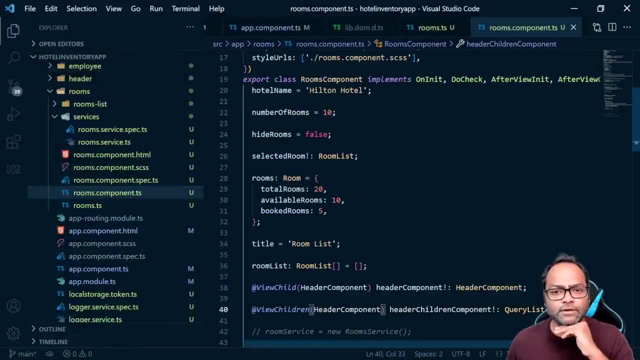 What we are going to see now is: We are going to create. We are going to create an observable by using RxJS itself- not using HTTP- And see how it works. So let's go back to our code base And let's create an observable by R1.. 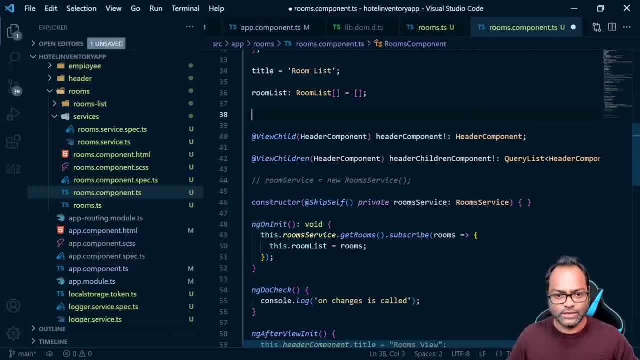 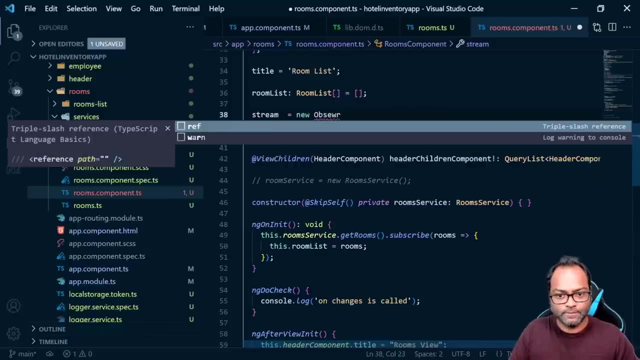 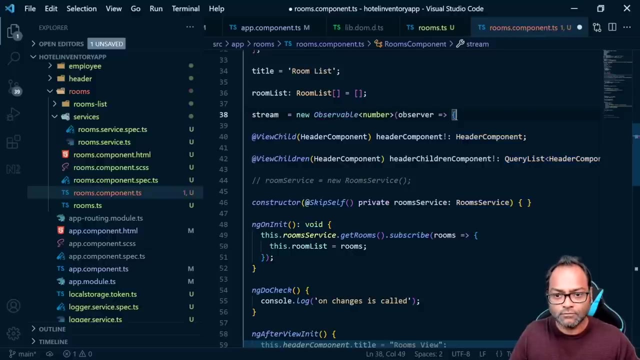 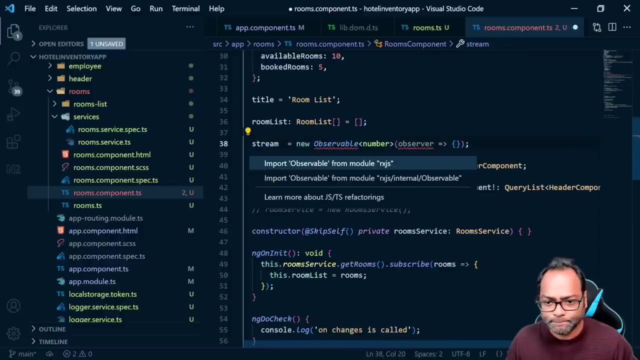 So what I'm going to do is I'm going to create an stream. I'll call it as a stream Is equals to new observable. Let's see, observable is something which should come from RxJS. Okay, It is not imported. 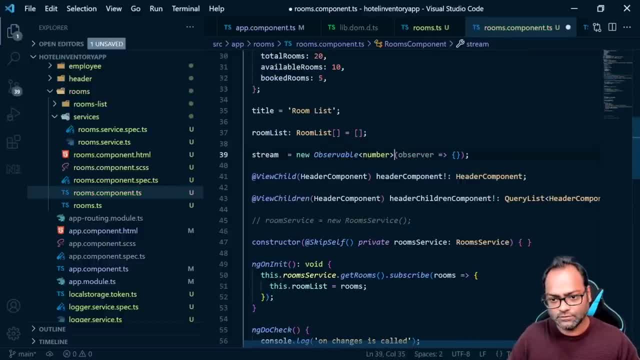 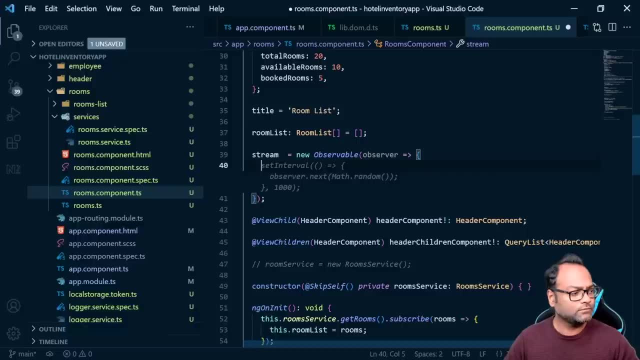 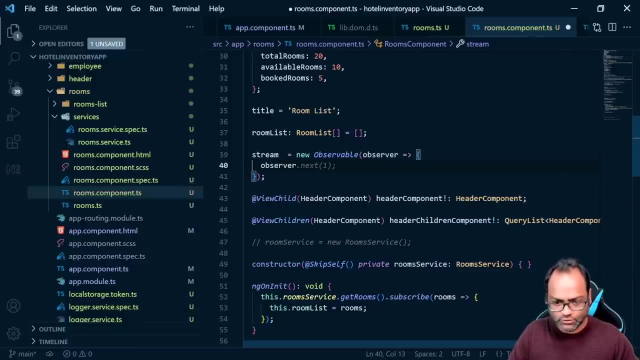 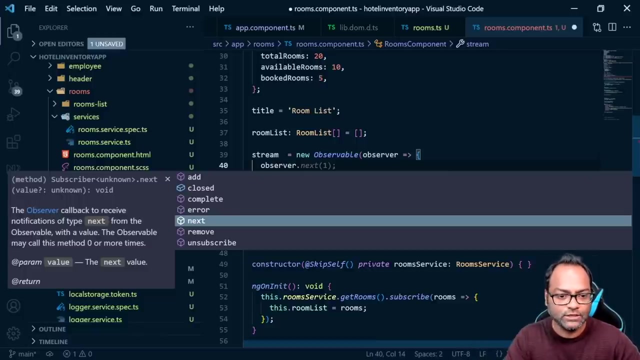 And it will remove this right now. Okay, And now, here in observe, we get an observer which we will call a method, called next. So there are multiple methods which exist on your observable. So you have, you can see. you have unsubscribe. 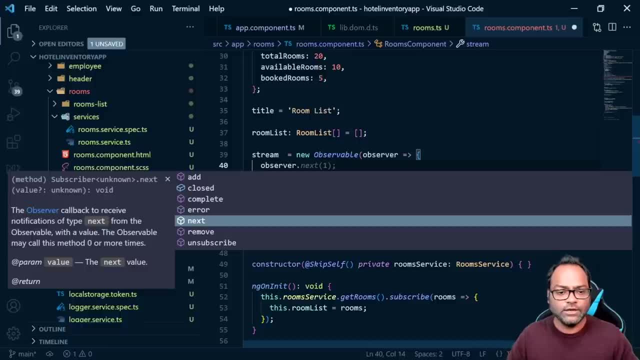 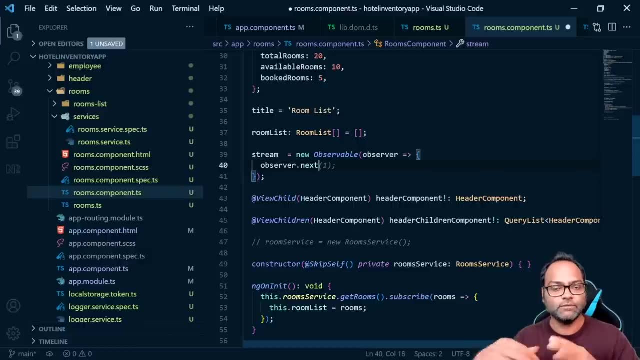 You have complete, You have error, You have remove and add. Here, what we are going to do is we are going to call next. What do you mean by next? So whenever you call a next on your observable, it will be emitting a new data. 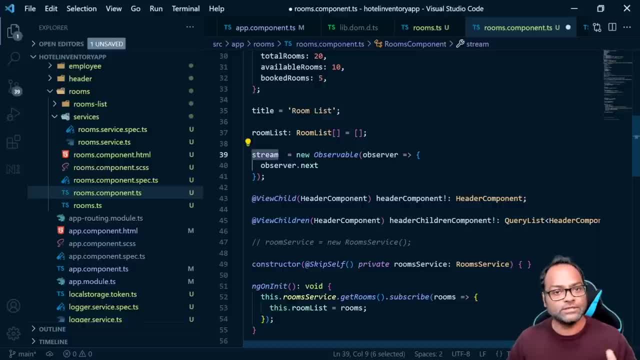 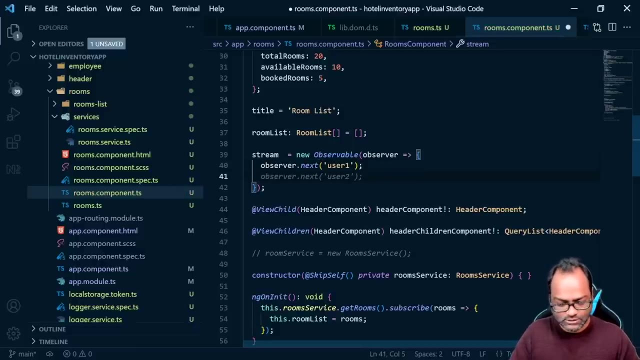 So whoever is subscribing to this stream will get this data. So let's say I'm saying the next data is user one And I can of course call it multiple times, So I can say, okay, this is observer dot. next user two. 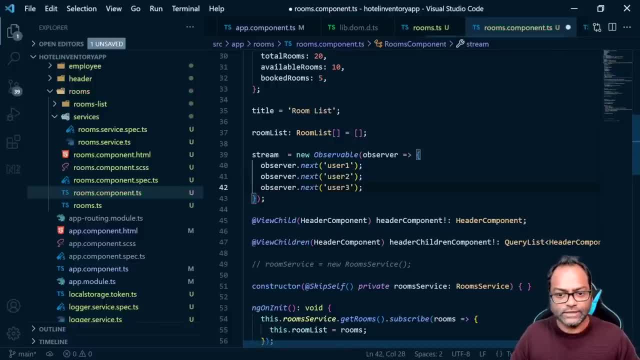 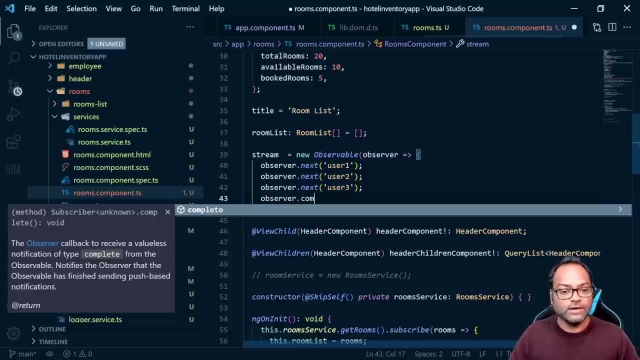 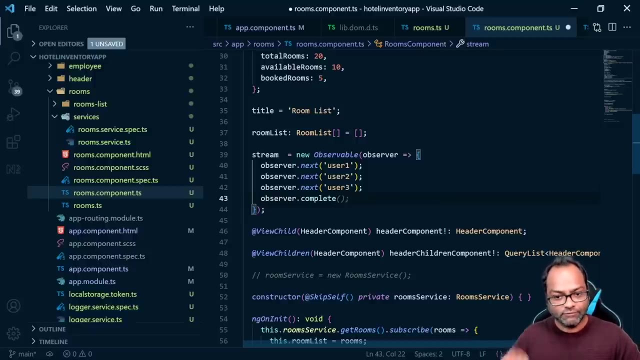 And next user three. And I can also call observer dot complete. Okay, So whenever this, of course every stream will finish somewhere. So I'm saying whenever this, after this, just complete the stream. So you can see I'm going to call complete method. 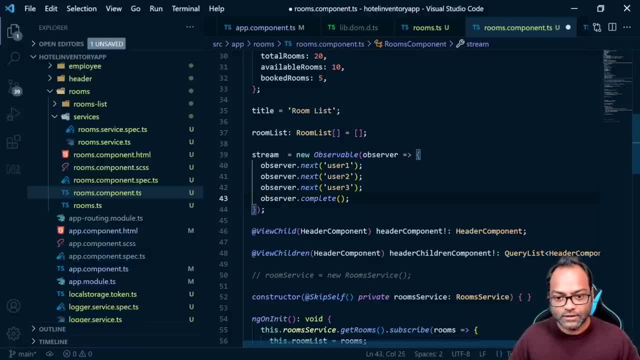 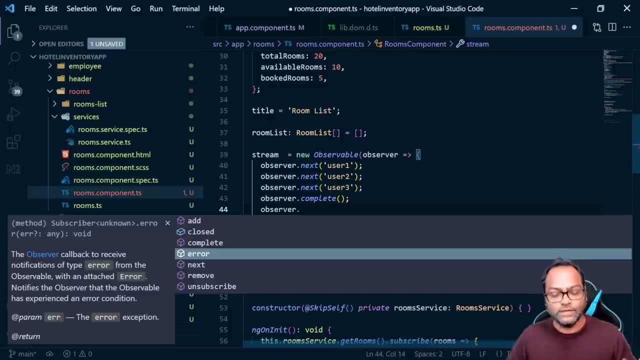 And this is where my stream completes, We can also handle. So you can see it says observer dot. We have one more method: error Right. So we can also handle the error in case. what if error? There is an error. 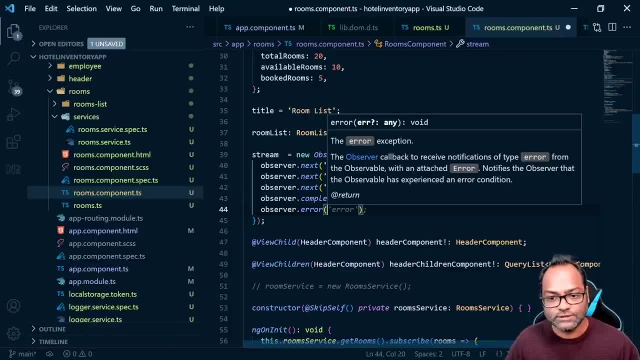 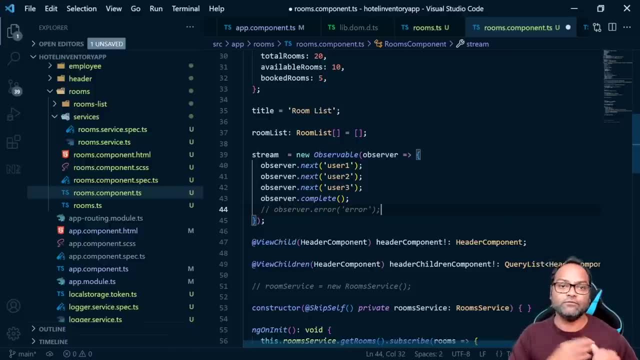 Right, So we can just say: okay, in case of error, just raise an exception and that's it. So we'll say this: I mean we are not going to use it. We'll see it later on, whenever a stream raises an error, how to handle those. 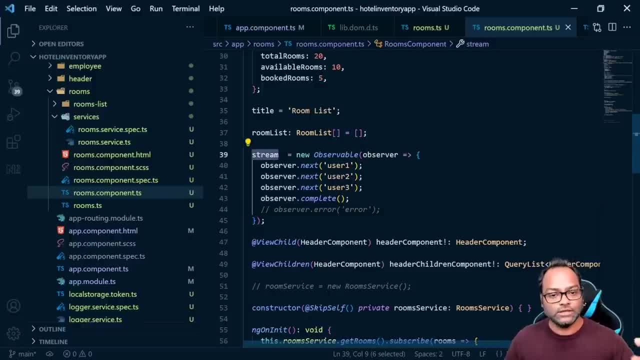 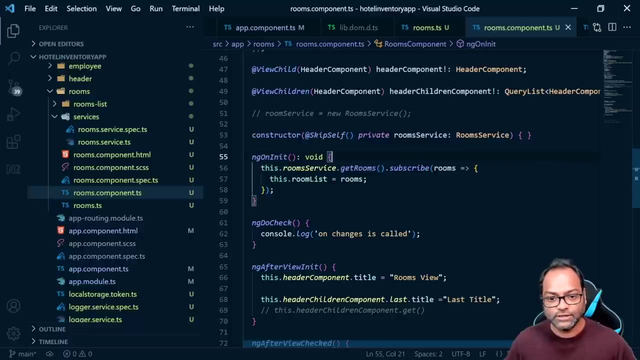 So we'll see that as well. So now this is our stream, which we can subscribe to, which has an observer and which can raise or which can give you a new stream every time you're calling it. So let's go to stream. ng on init. 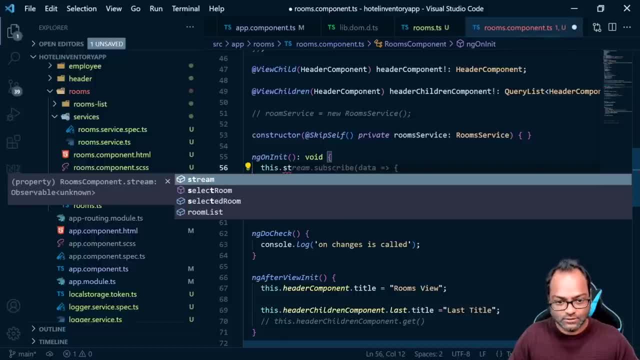 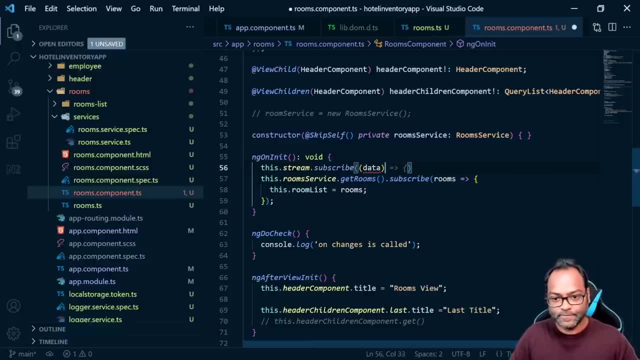 And here I'll say this dot stream And we will subscribe to this Right. So we'll subscribe and we'll say this is data and we'll call console dot log and we'll see what the data is. Let's go back to our hotel inventory app. 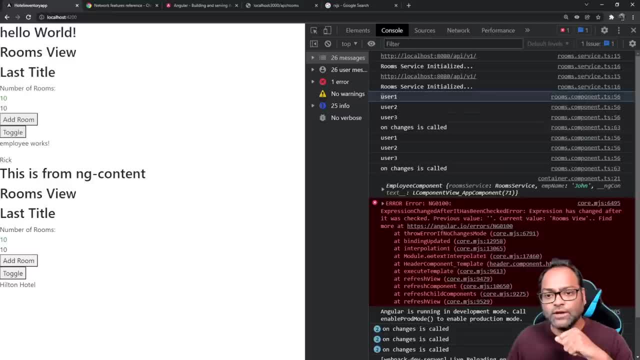 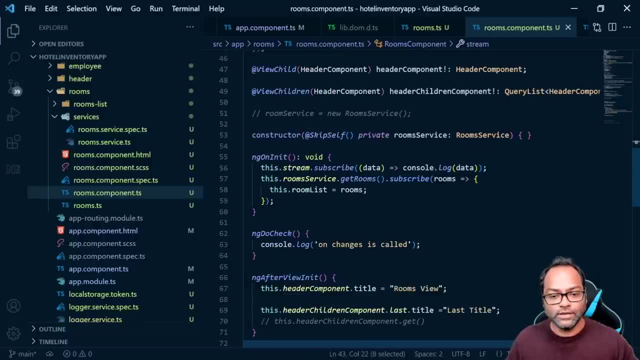 Let's go back to the console And you can see you have user back. You can see you have user one, user two, user three. After this, your stream gets completed. Right, So we are calling complete. Let's try to call this again. 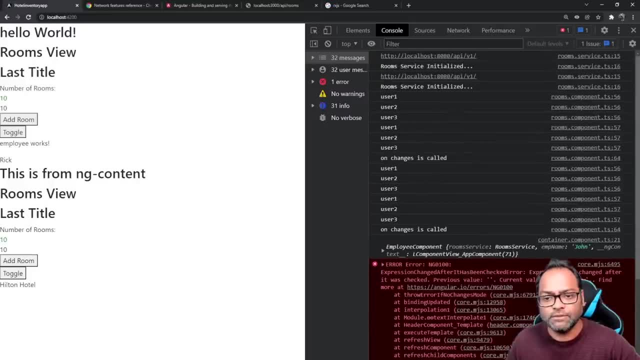 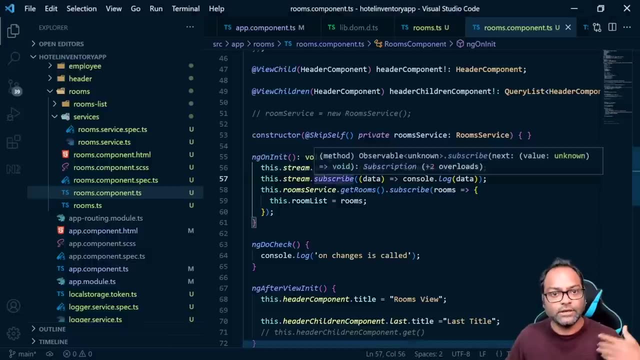 So we are calling it multiple times. It is anyways happening multiple times right now, So you can see user one, user two, user three And again user one, user two, user three is getting rendered. So we are subscribing to the stream multiple times and we get the same data every time. 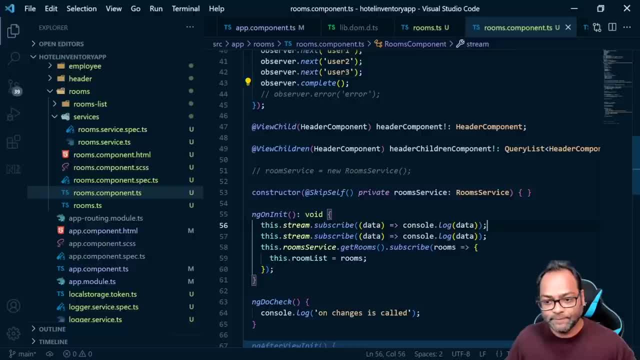 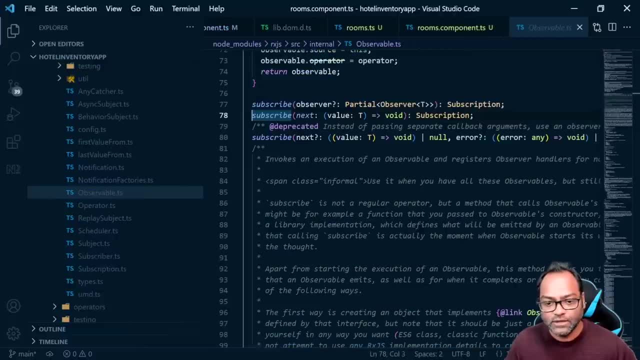 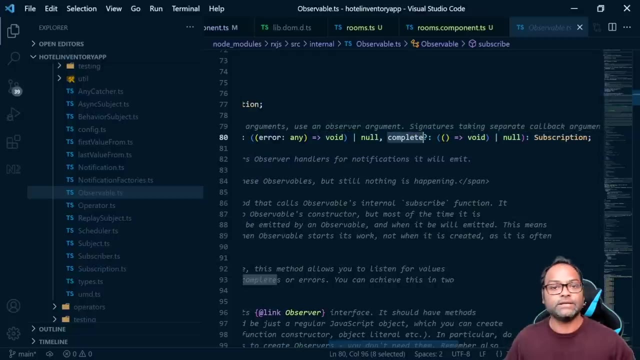 And after this your stream completes. Inside this subscribe also, you can get three values, So let's go ahead and see the definition, of course. So you have next value, You have error And you have complete Three values. 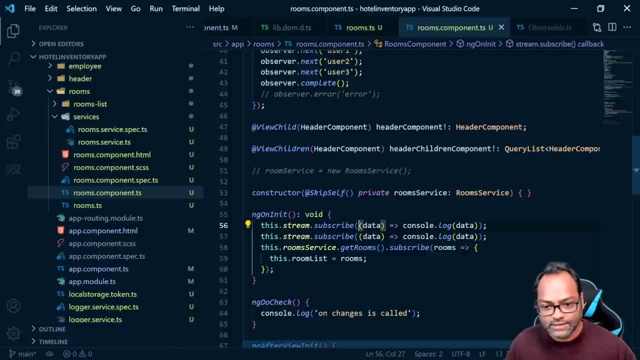 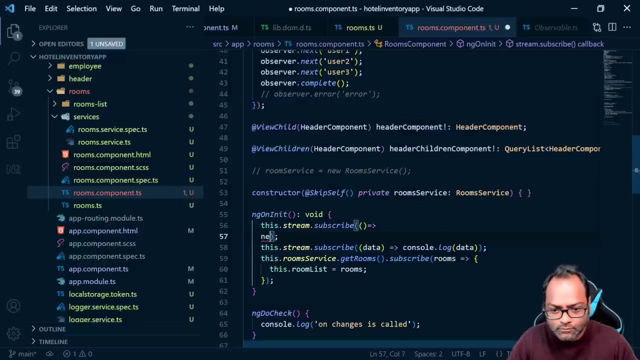 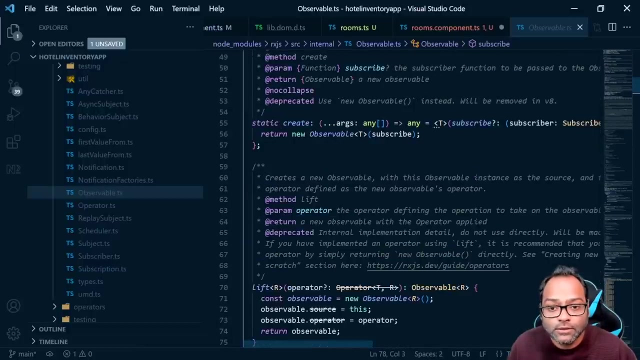 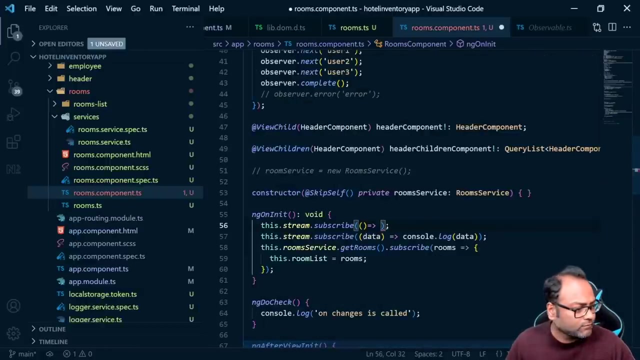 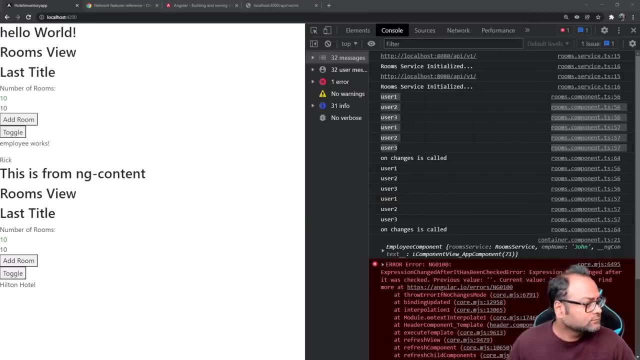 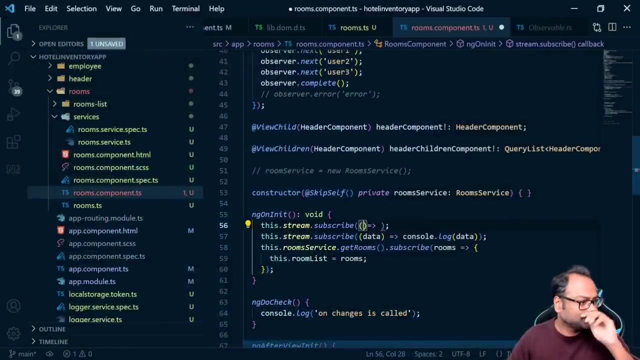 So you can actually write this, as This is our next value. So it's okay, Okay, Okay, Okay, Yeah. Is that somewhere clear? So once we subscribe to this, we get three types of data, So you can see we get. 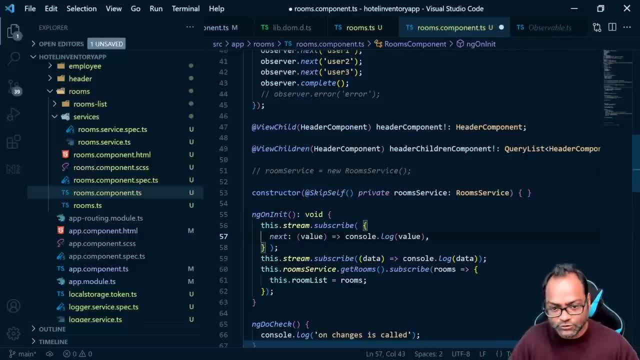 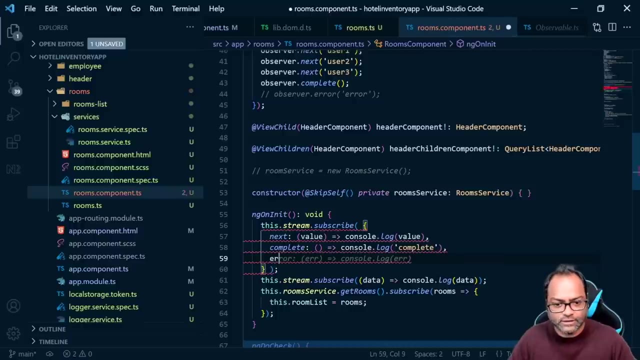 next, which is of course next value. So we can also do something like this: On complete, I am going to say: just go ahead and complete, We'll just print that this stream is completed And in case you get error you can also just say okay. 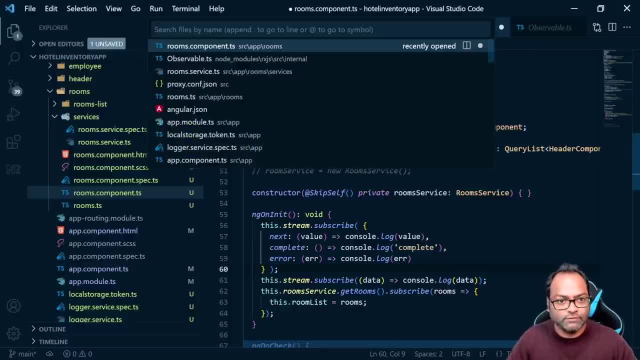 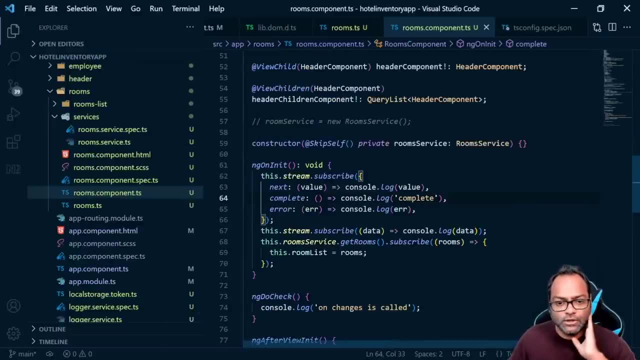 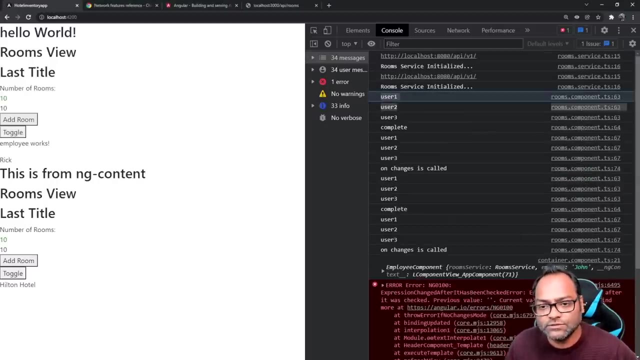 there is some error. So, whatever the error is, you can just print it. Let me just format So we have next complete and error. Let's go to our UI again And you can see it says user1,, user2, and this is where your 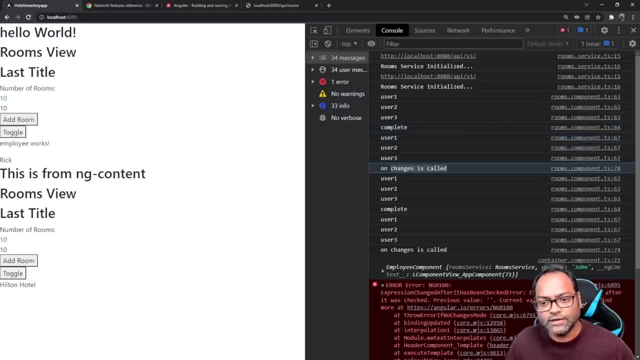 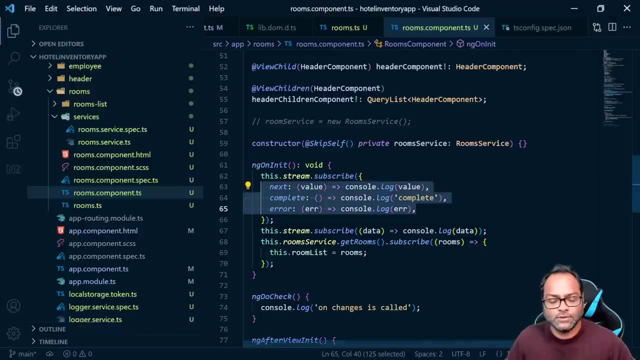 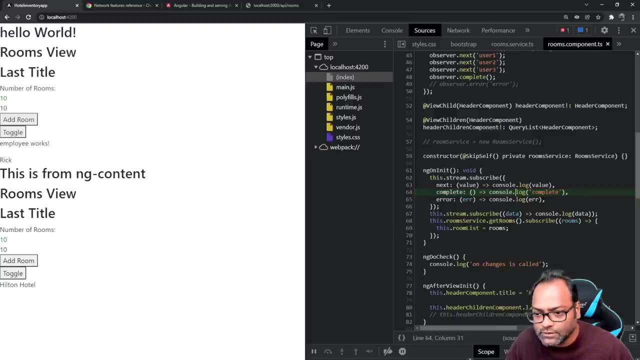 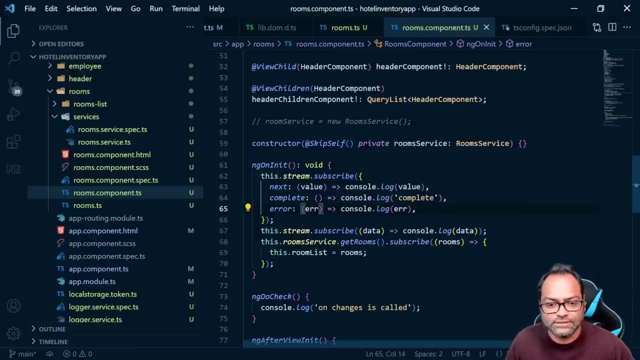 stream completes, Then again user1,, user2,, user3, and your stream completes: Okay. this is at another place where it is getting called So user room component. This is the one. Okay, because our rooms component is getting rendered twice. it is getting called twice. That's the thing. 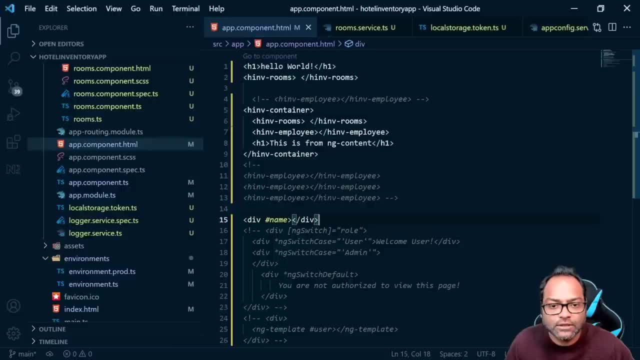 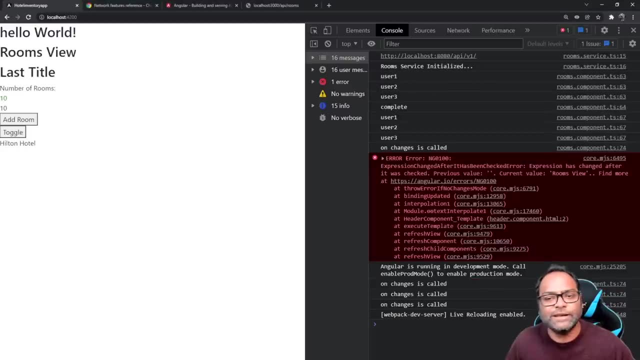 I think it has to do with this. So we have portal rooms here And let's comment this one. So we will just use this And it will be rendered only once. So you have user1, user2,, user3. And then it is complete. 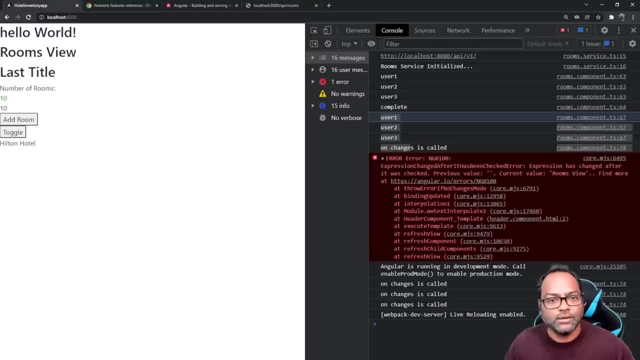 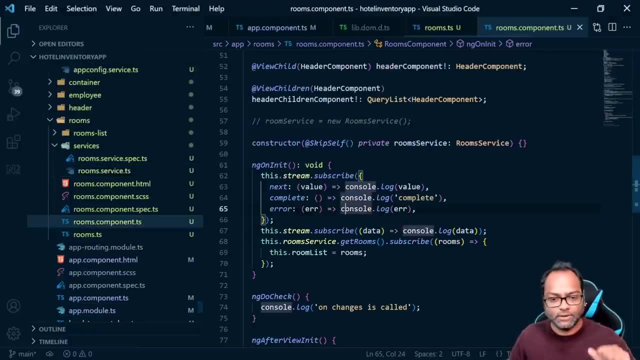 And then you have user1,, user2,, user3. And then your stream completes. So this is what will happen. This is what we will be. we won't be using this syntax. We will be using this syntax a lot of times, Even not. 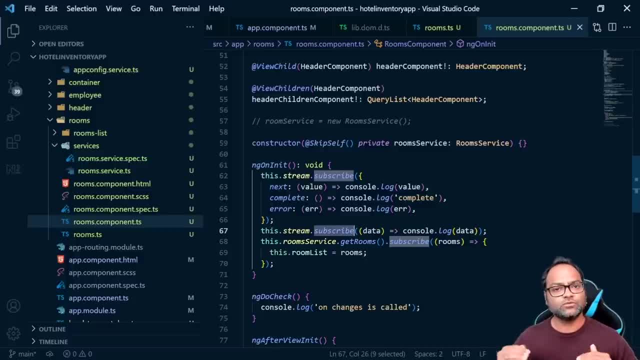 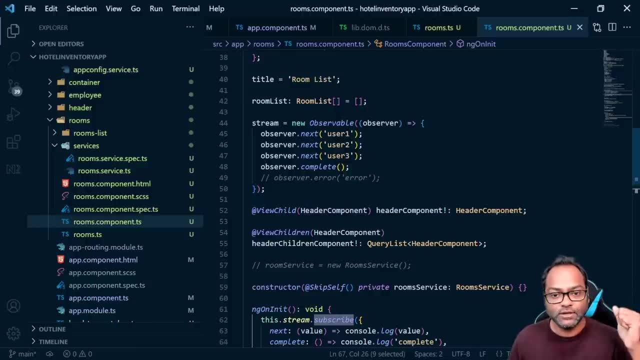 this syntax, We will see what is the standard way. This is just to make sure that you understand streams. So what we have as part of streams is there are two parts. One is, of course, your observable, which will be subscribed, Which your users can subscribe to. 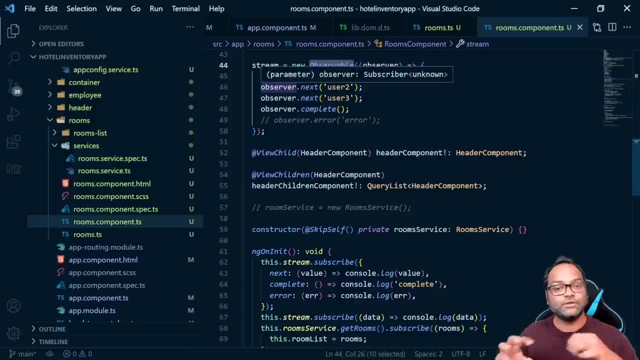 And internally observable, will have an observer which will observe the data if there is a new value which is available Now where this is useful. So in case, let's say, you are working with some real time database, So whenever a new value is like, pushed because 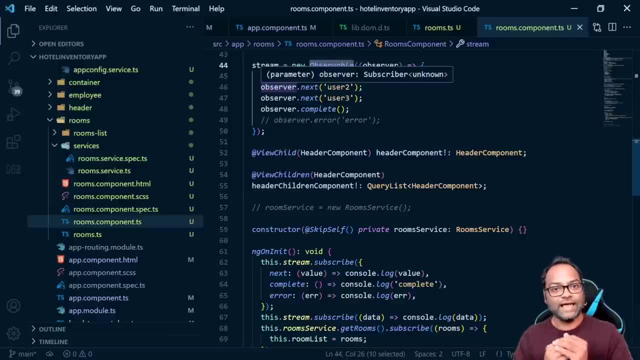 it's a push based architecture. Your observer will actually observe. okay, there is a new value, So what I have to do is I have to call next Internally. this is what it will be doing Internally. it will call next method. So whoever has subscribed. 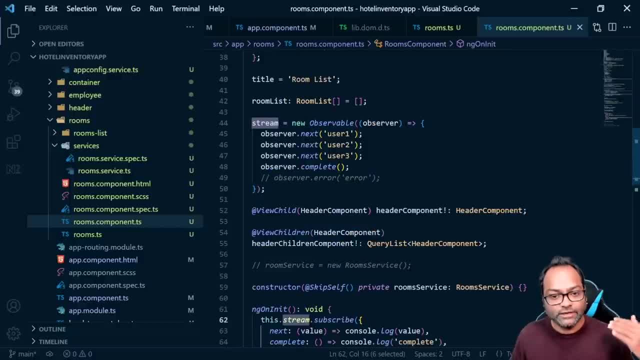 to, it gets the new value, Even in case it also has complete and error. So in case you get some error or your stream completes, that's it. If your stream completes, it will not going to give you anything. In case error is sent, it will. 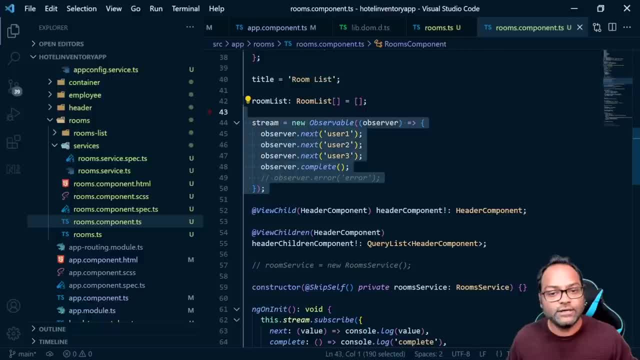 capture that error and it will send it to you. You don't have to go ahead and create this by your own. You will be using some operators. of course, we will go ahead and see that. This is just to let you know how observables internally work. 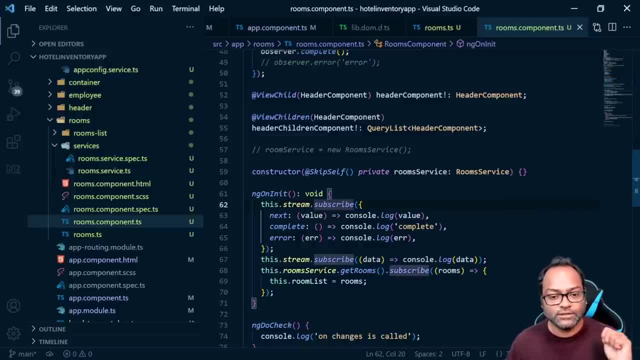 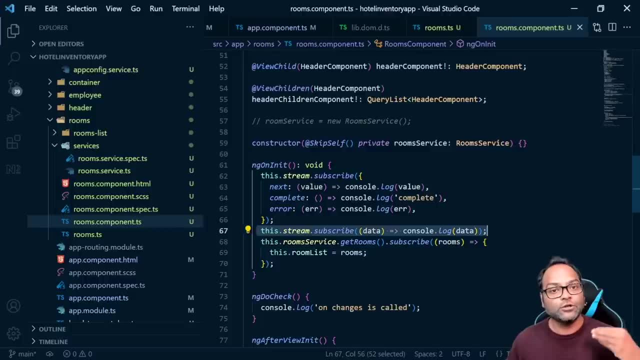 And what you get once you subscribe to it. You get next complete and error. These three methods are given to you. Generally, what we do is we work with data, But you should also work with. try to handle the errors gracefully as well. I mean, your users should not see. 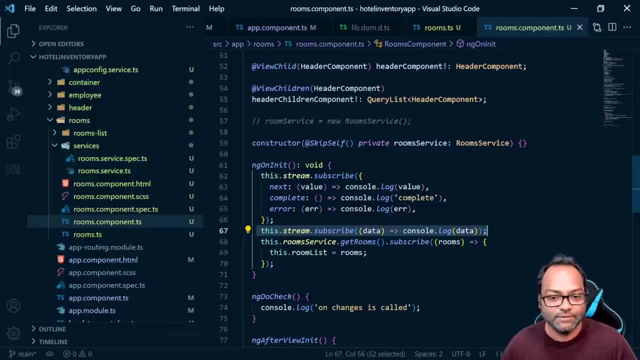 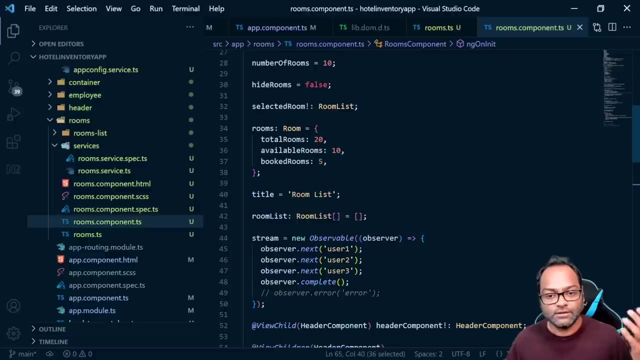 the error Red lines once your application is available. So we will see how we can also handle error in case we get it from the API. So this is all about observable streams, Observable observer and how you can create it manually by using observable class which is available here. 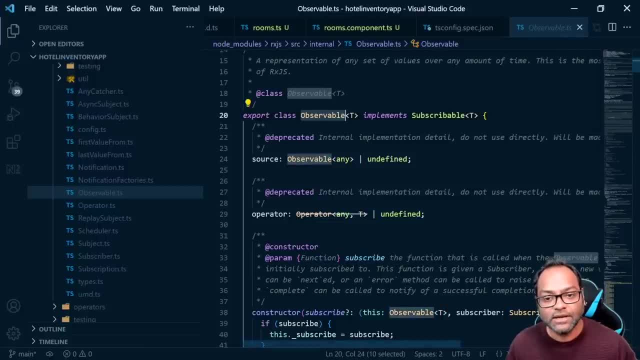 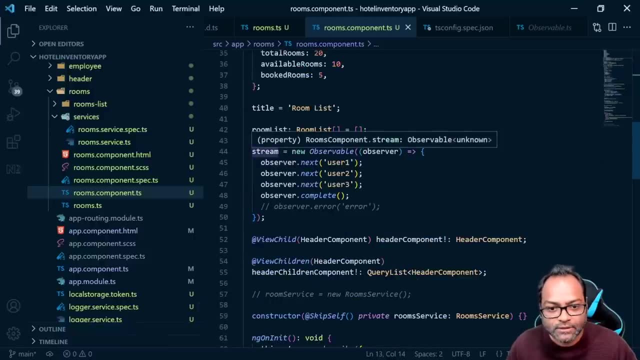 So if you go to this rxjs, observable, you will see this is a class And it also has time. So right now, if you see, let me just show you here. So it says: observable of unknown, because we have not given any type We can actually make. 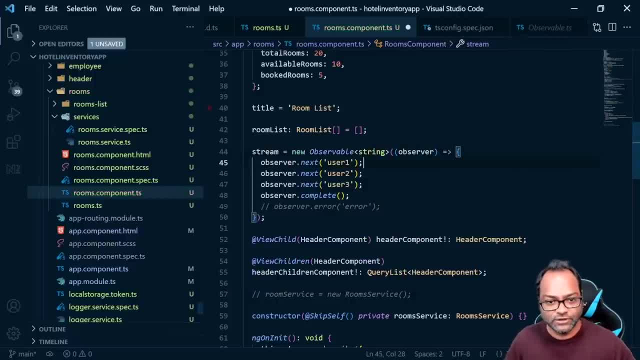 it string, because right now I am working with string, So it will know. okay, this particular stream will have string of data. You can make it number, in case you are working with number. But yeah, this is higher level API. You don't have to do it. You don't have to use it directly inside your code. 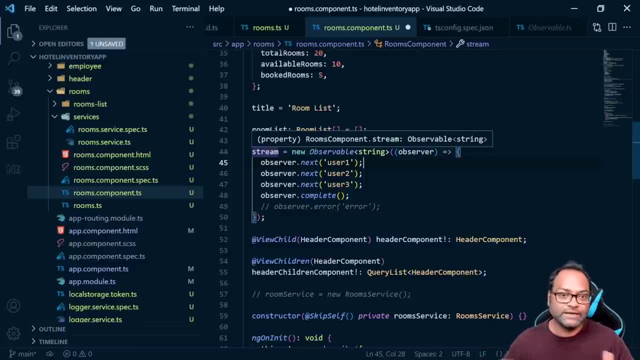 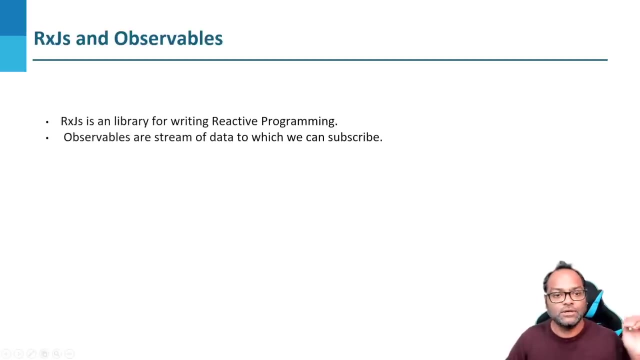 Because most of the time, you will be using http and you will be getting the data from there, or you will directly work with streams by using other methods. So we will see those Right now. this is what we have in rxjs and observables. Now let's go ahead and move into other methods. 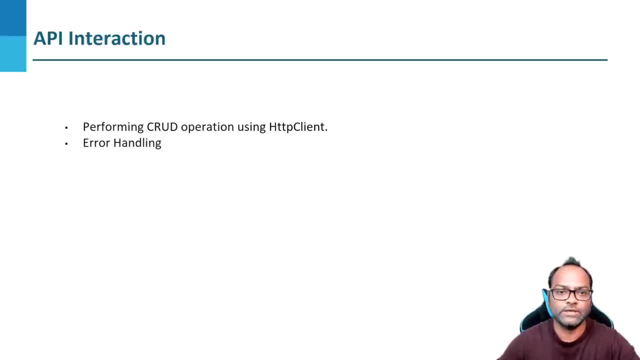 Move on and see other operations. Right now we have done get operation and we discussed something about rxjs. Now we will. next we will try to do post operation. So we are done with read, Let's do it. Let's see create and let's. 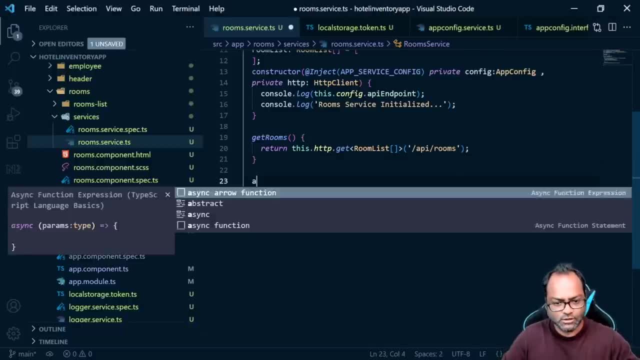 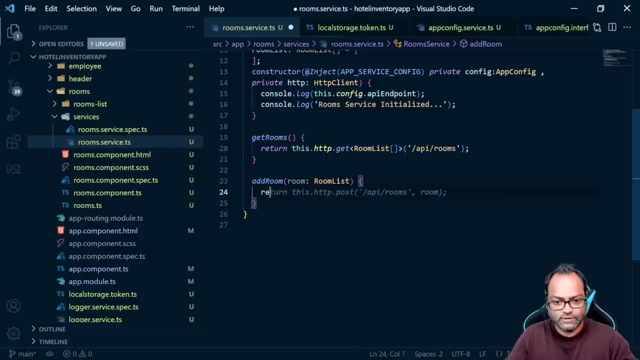 go back to our code. This is our service and we will call add rooms. Okay, we will pass one room, not rooms, and here we are going to do return thishttppost api, slash rooms and the room data which we have available. So our service is done, This is. 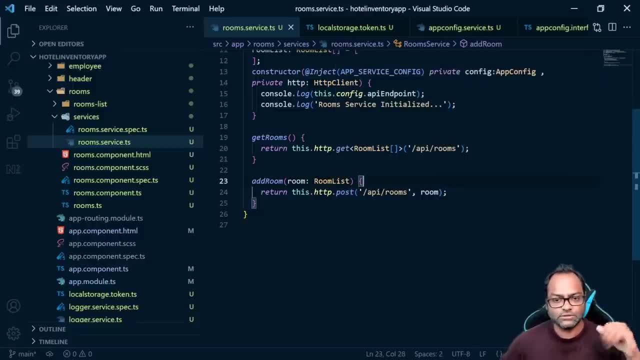 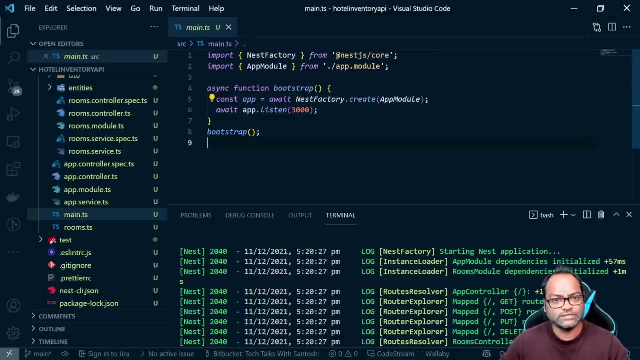 the service is done. So this is it, But you have to be aware, whenever you are working with APIs, you should be aware of request format as well as response format. So let's let me just check what is the request and response format for my this particular API. So we have this post. 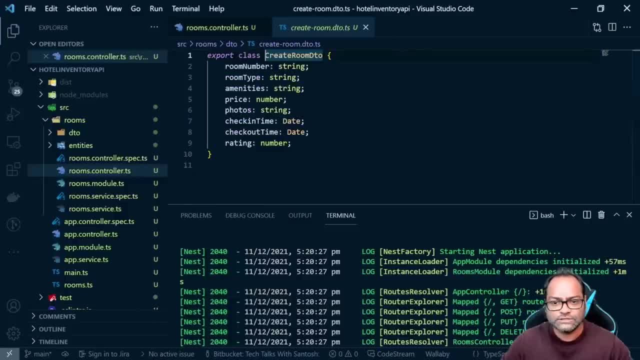 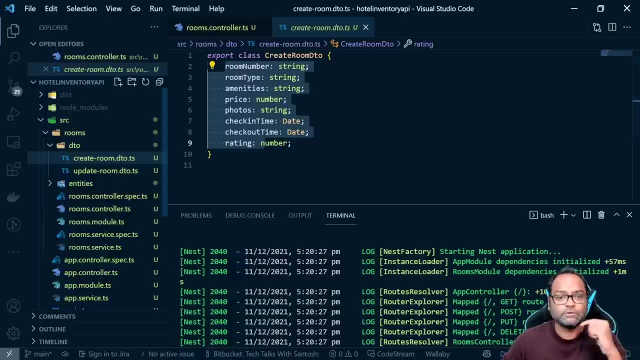 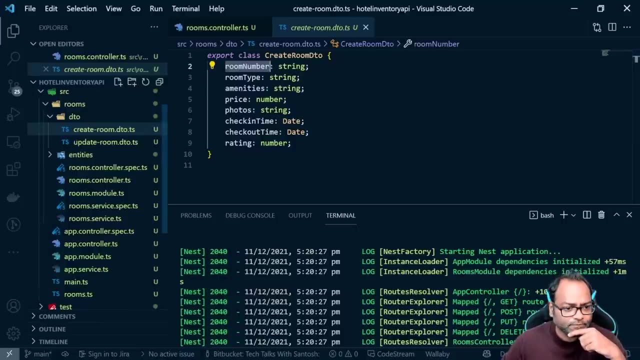 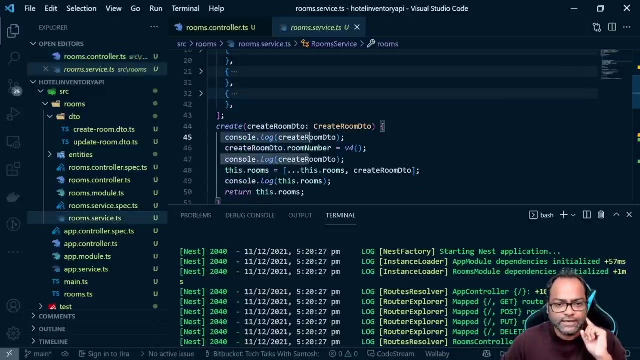 This is the create and create room, which is which requires room number, room type amenities, everything apart from the room number Which will be created for us, And let's go ahead and see the service Just to see what will be the response. So, in create, this is just. 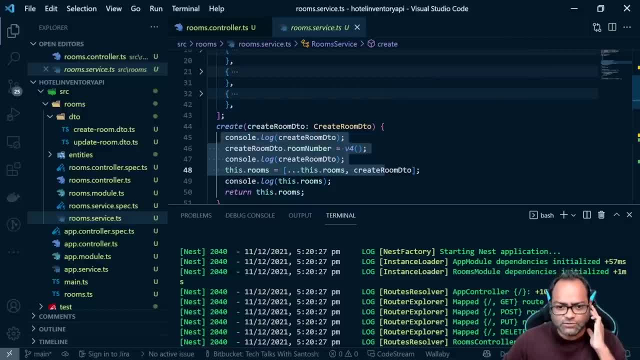 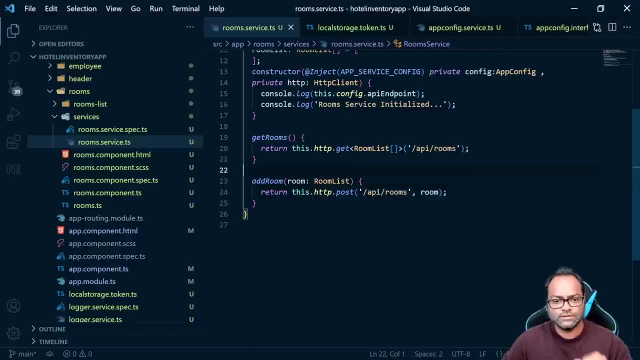 of course, I am not accessing any database. So, okay, I am returning the rooms entire list of data, which is which is added now. So let's see, So we have this post. Generally, you get the latest record which is added, But it's up to you. I mean, it's a really bad practice. 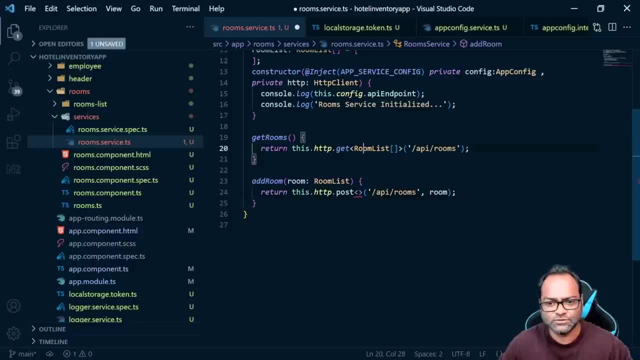 to return all the data which is added, But this is just an example, So I am just going to return all the data which is available after adding this record as well. And now let's go back, and this is our add room function. You remember? we just wrote this. 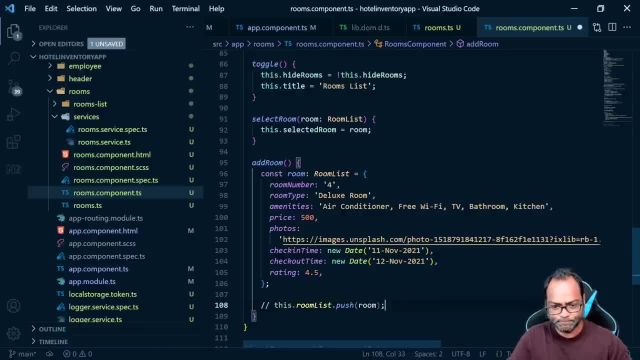 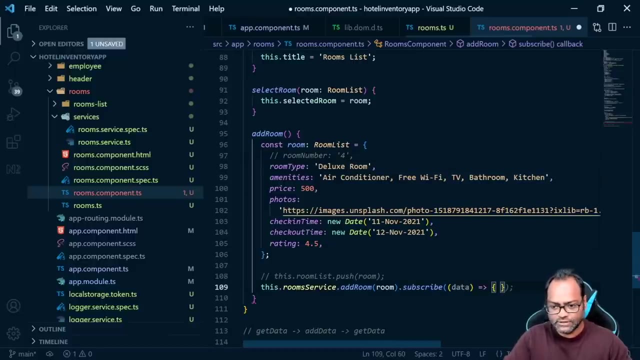 here We will call comment this and we will say this: dot room service, dot add room And we will pass this room as the data. I will comment out room number which won't be passed yet. Let's see if it gives us any issue otherwise. 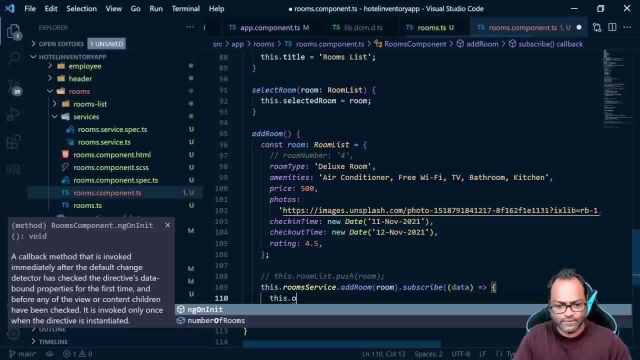 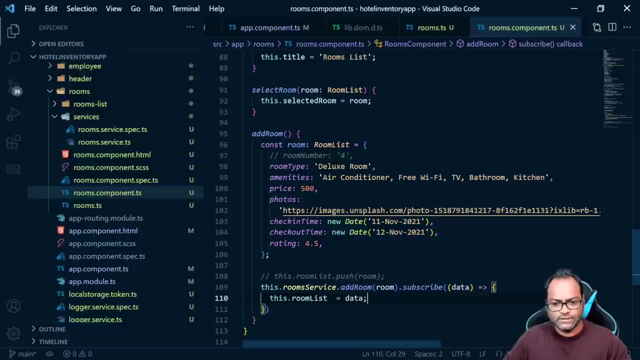 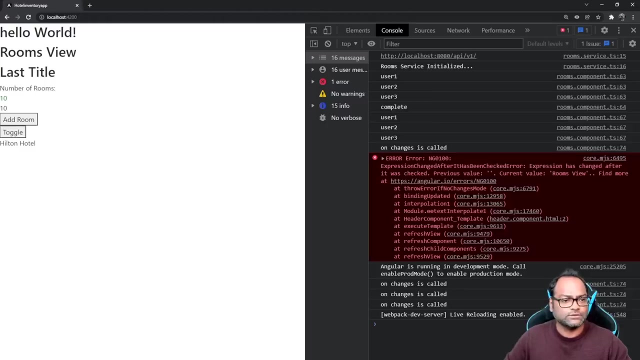 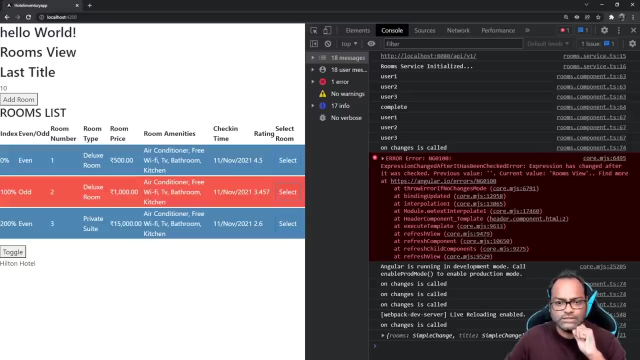 this should be fine And this dot room list. we will assign whatever data we are getting from this response to room list. So we let's go ahead and try to let me just close other browsers and we have our get data. So this is available. Get call succeeded and we. 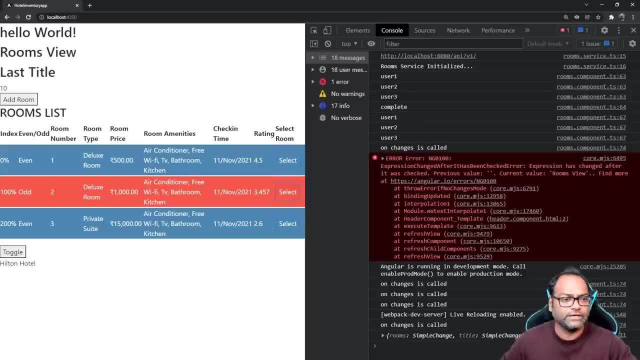 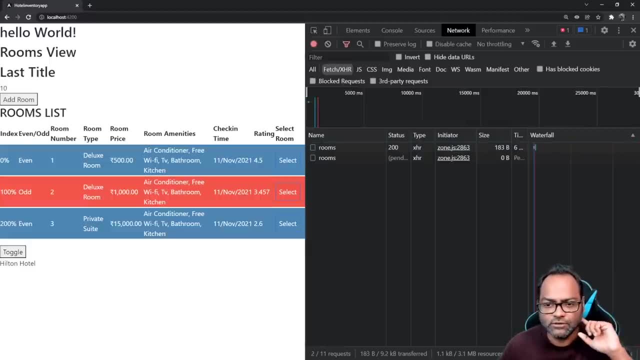 got our data from the API. We want to test add functionality. So let's click on add room. Let's go to network first, because this is where we will be able to see our request. Click on add room And we got 201.. So, if you see, 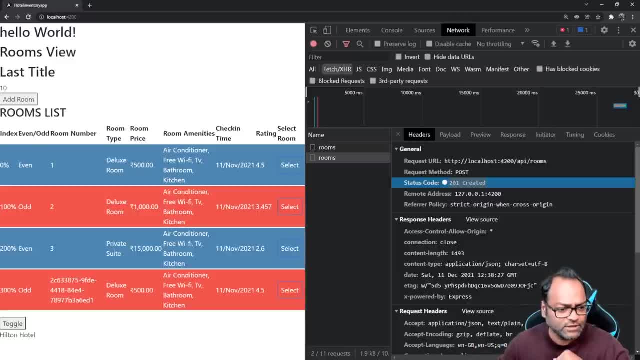 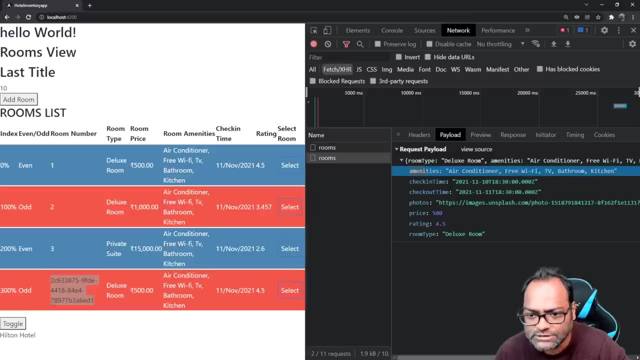 we have 201 created. It means my API was successful. We also got the latest record, which is added here. You can see, the ID is alphanumeric because it is generated using UUID, which will be unique ID And it's alphanumeric string. So let's see the payload. So this is the payload which we have sent to our 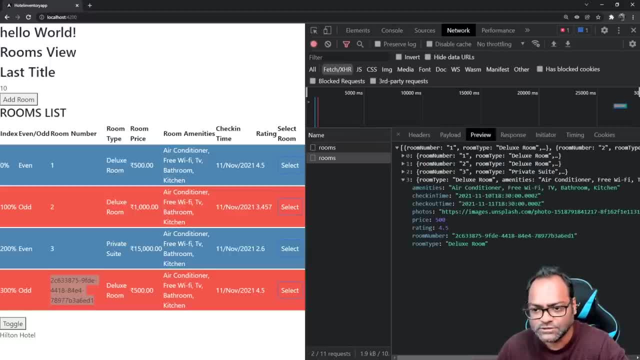 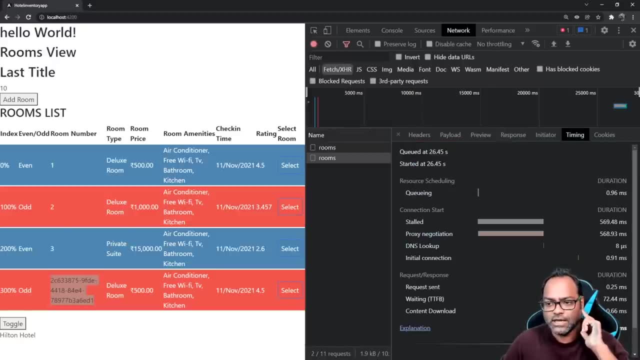 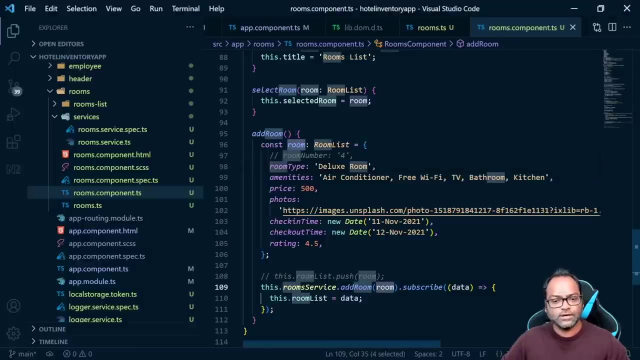 API And, of course, this is the response which we have received And this is JSON response, in case you want to see it, And you can also see other information. So your timing and everything. So this is it, This is how you make a post call, I mean in case you get a single record, of course. 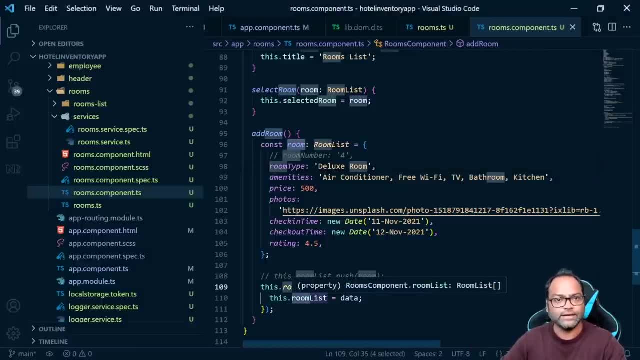 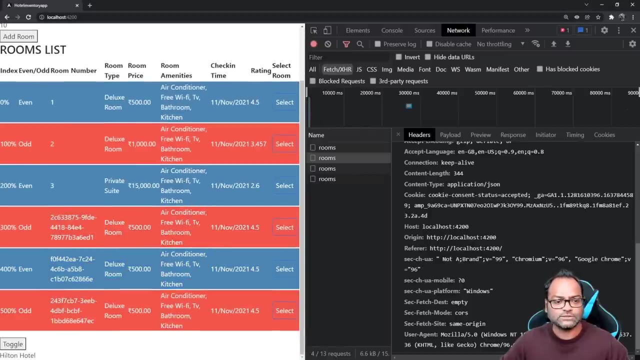 you have to go ahead and see how to handle that data, But right now I am returning all the record, including the current record. So I get everything which is available And I can add more So you can see. So you have these different records. 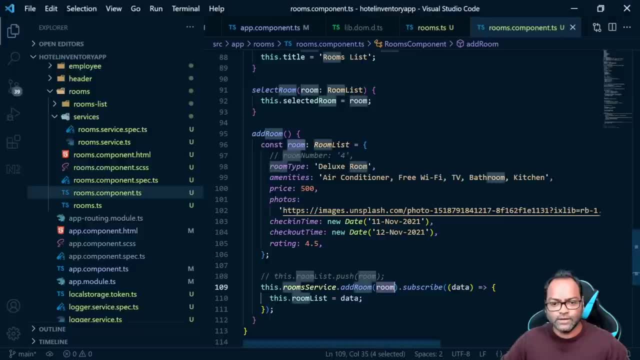 with different ID. The same record we added with different ID. Right now, we have hard-coded the data because we don't have any form. In future, we will replace this with a form. That's what we are going to do, So let's move on and make our next API call, which is now: 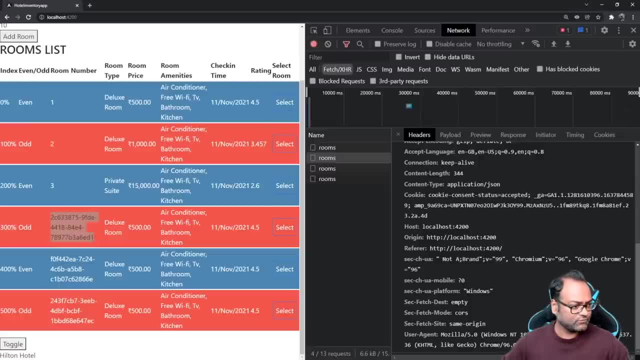 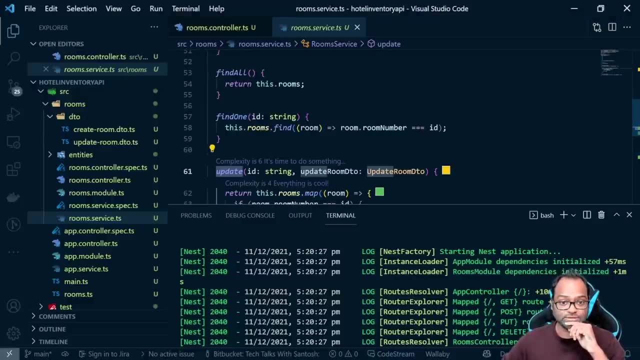 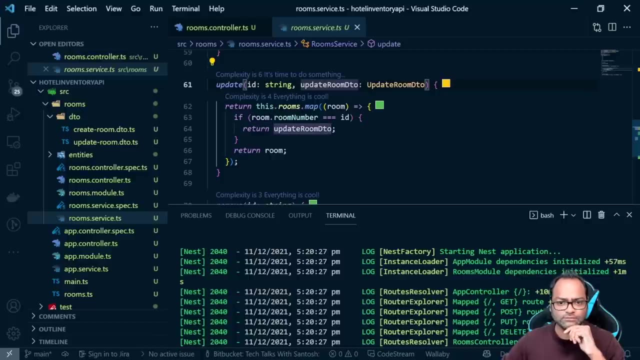 update. So let me just check quickly what is the update API looks like. Okay, So this is my update And it takes the data and updates the data and gives me back. Okay, Let's try to make an update call, And here what we are going to. 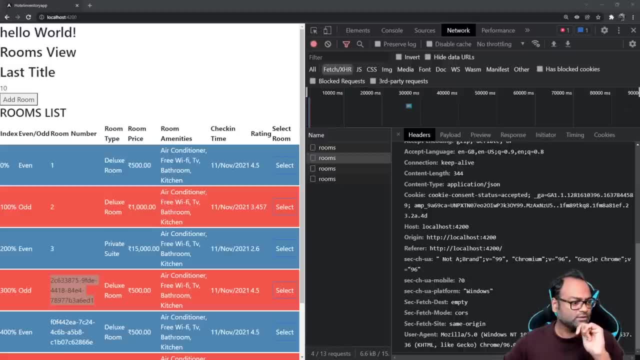 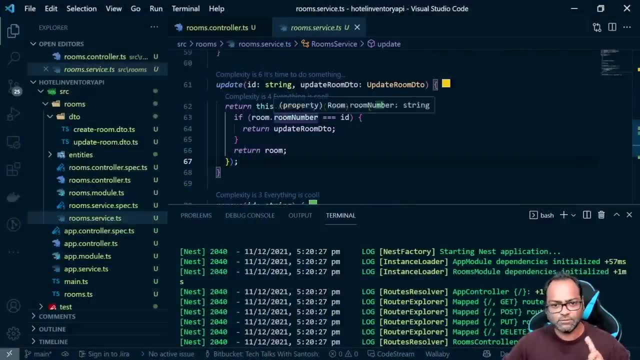 do is, Again, I am going to hard-code some data Just to see how to make this call, And this also returns the entire records. Remember this: This also returns the entire records. In reality, you are not going to get this. You are not going to return entire data. 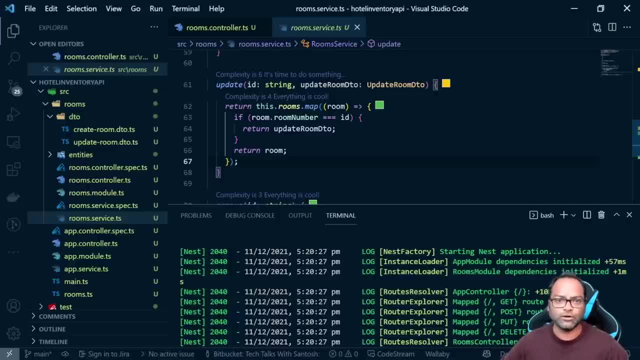 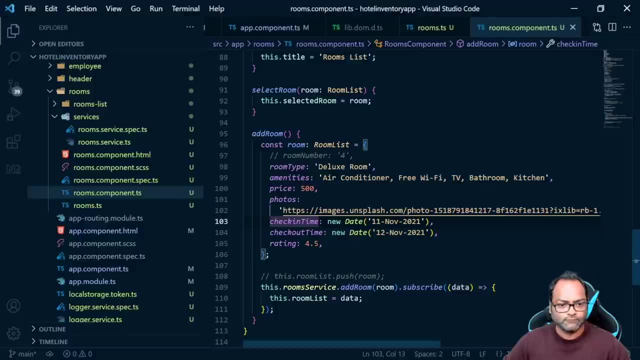 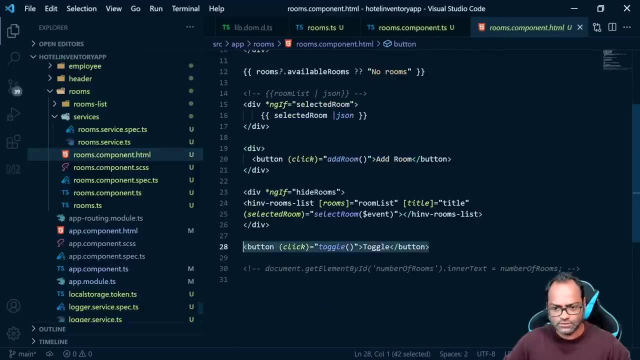 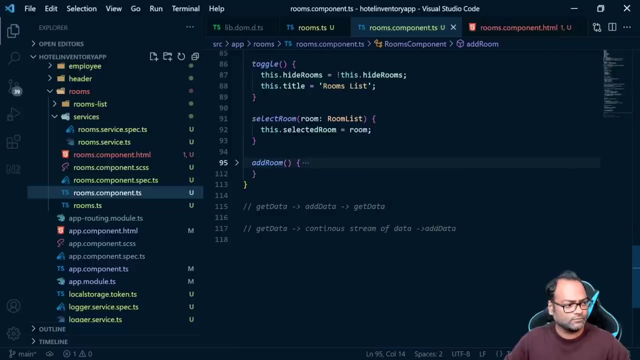 Probably you will get the ID Right. So this is updated or not. That's it. So let's go ahead and add a button And I will call this as edit room And let's implement this function. Okay, So edit room function. 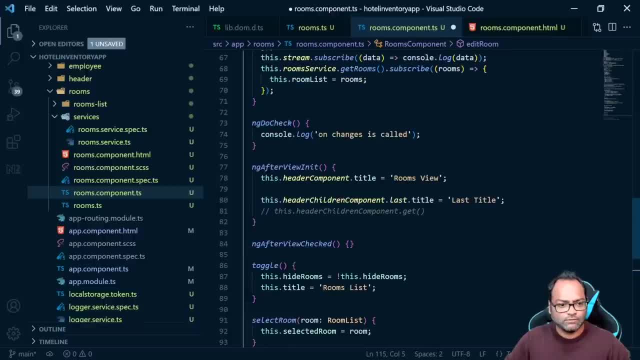 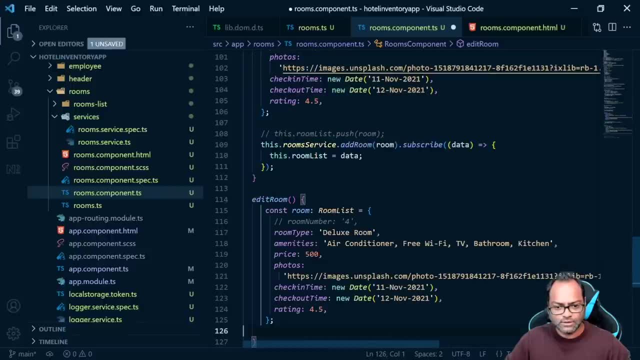 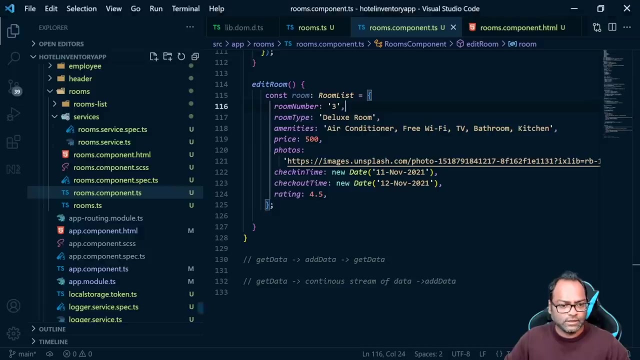 And, as we said, we are going to just use the dummy data here as well. So I will take it from this And I will say room number 3.. So this data will be updated for room number 3. And we will call it as edit. 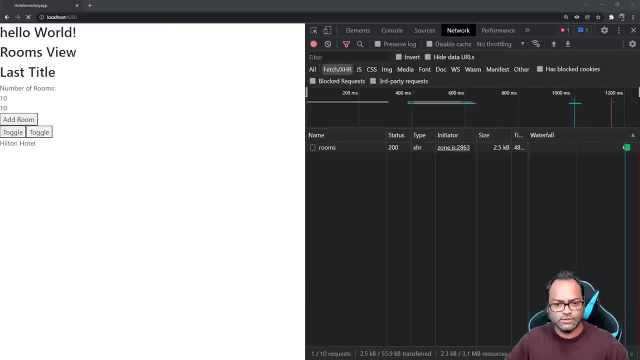 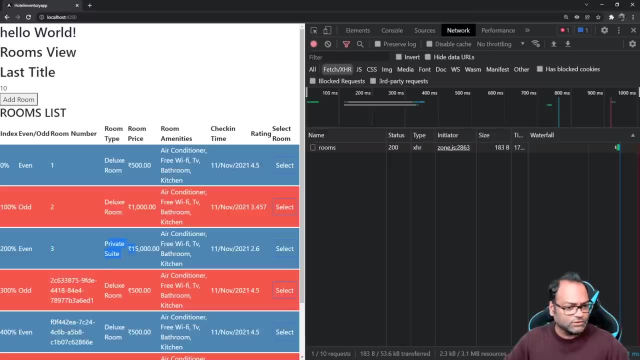 room. Again, in future we will have a form from where we can edit this record. So let's see what we have at room number 3., Which is private suit, and 15000.. So I think we have a different. Yeah, So we have. 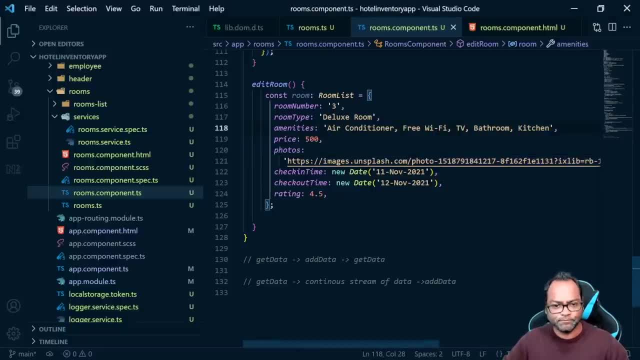 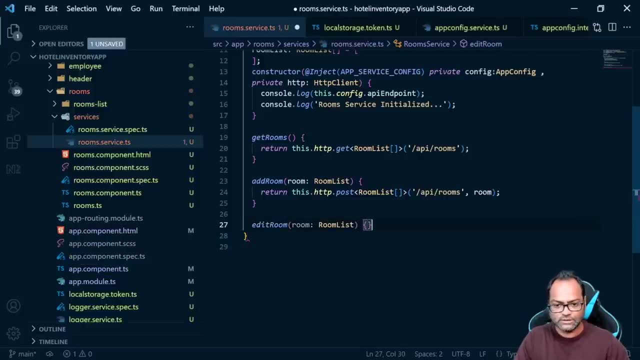 different record here, So this will be updated with room number 3.. Let's write the method. So I will say this is edit room, Which will get a room data And will return. So I will say this is httpput. 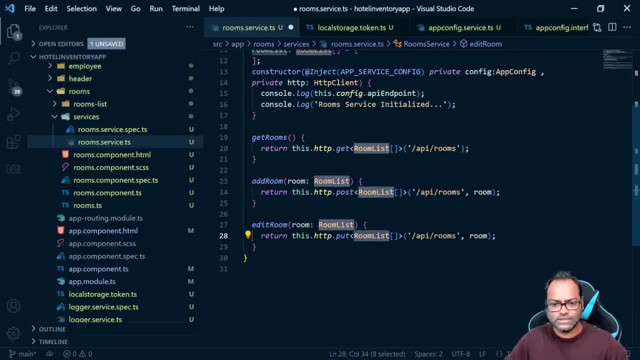 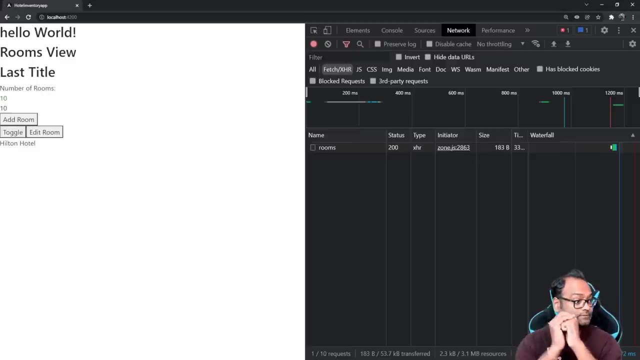 And again I am returning the entire list. So I am saying, okay, this is the type of response, And then edit will have the same API and this is our data. Let's go ahead and save this. 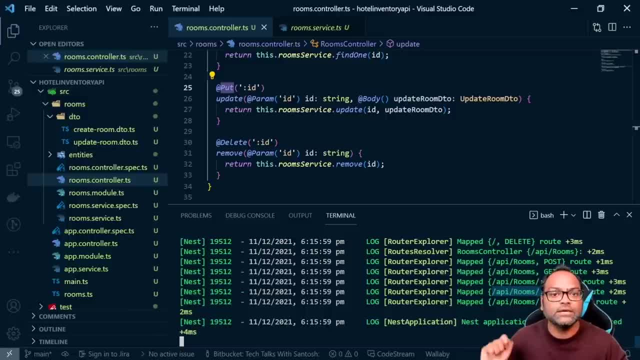 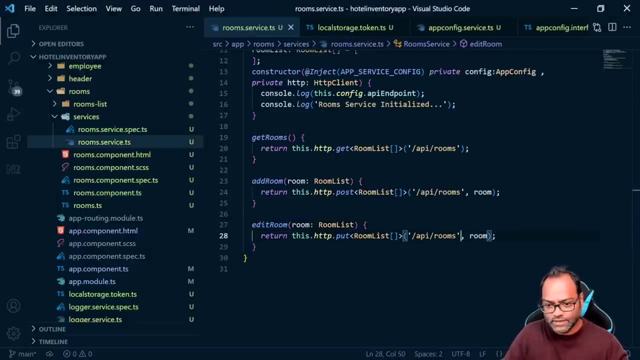 slash room slash ID. so we have to pass the ID in the request itself. so let's go ahead and see how we do that. so you go to edit rooms and this is where we have to pass room slash id. so we'll say, ok, I am going to use this, this tick operator. 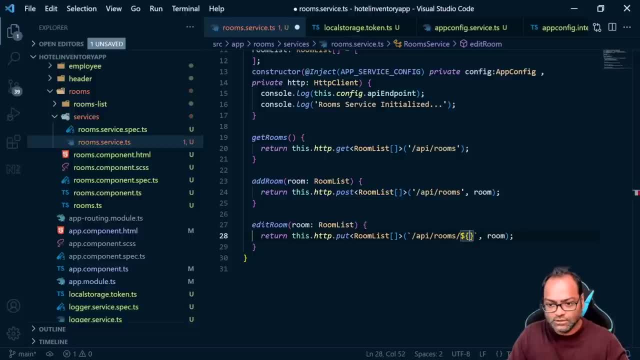 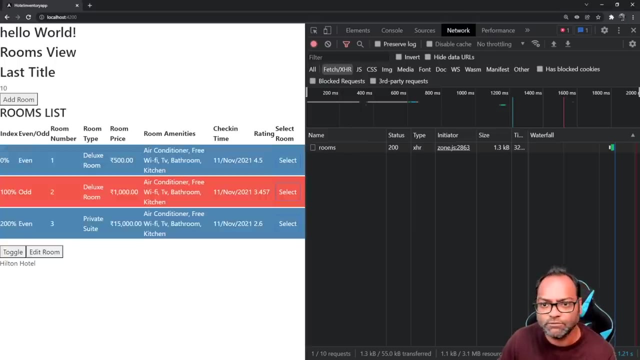 and as a slash dollar and here answer room or dot room number, which is the ID for us, and let's go ahead and see. let's go ahead and see. Let's go to the browser and see the data or see the request which is being passed. 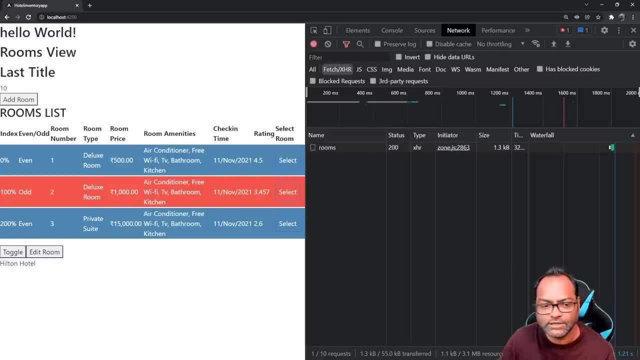 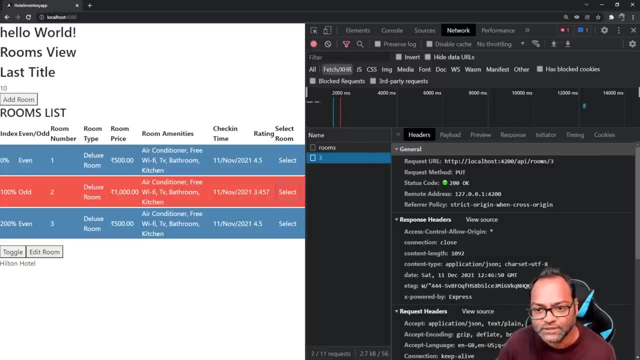 Let's click on. let's go to the network. We are already on the network tab. Let's click on edit room and we have 200.. Okay, Yes, we made our put call as well. So we have this payload and you can see the data is updated as well. 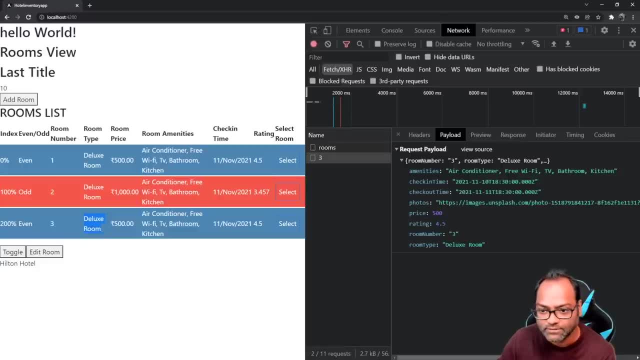 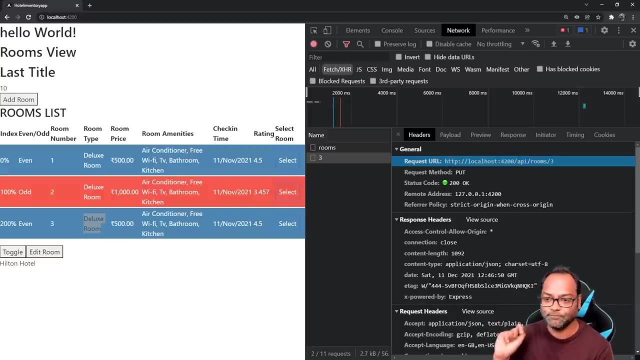 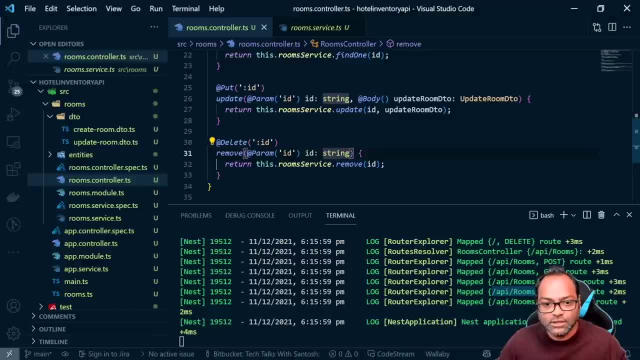 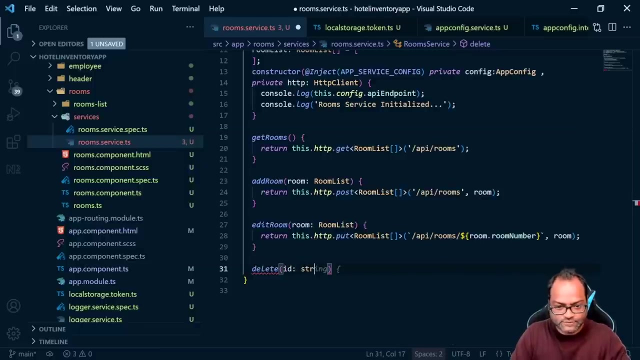 So this is how you can make a put call. So this is, this is: let's see the delete next. So I'll say delete And if you see, delete also requires the ID to be passed. So I'm am going to do is I'll say just id, just type of string. you don't need to send the entire data. 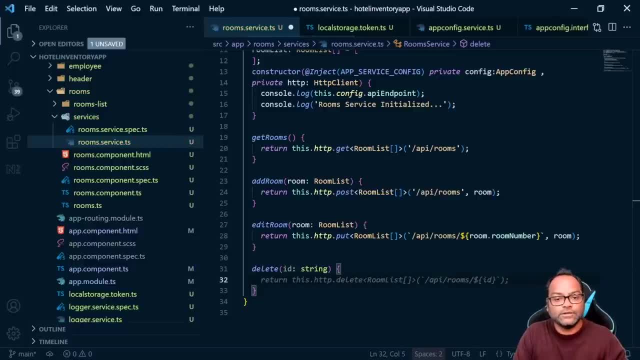 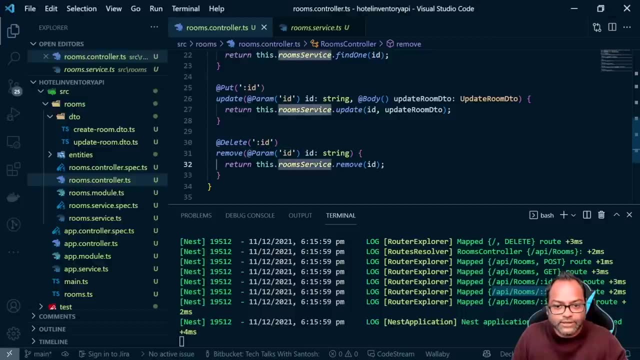 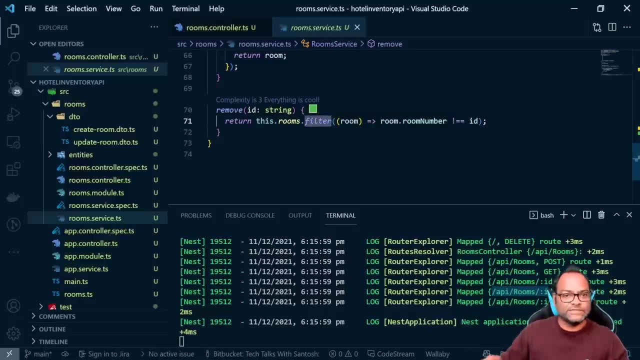 to delete. so, and delete also does not return anything. so you can see: okay, here, right now, it returns the id, that's it right. so it returns the. it returns the data apart from this id. we, as we said, this is a dummy api, so I'm returning all the data, but in reality, you will find that 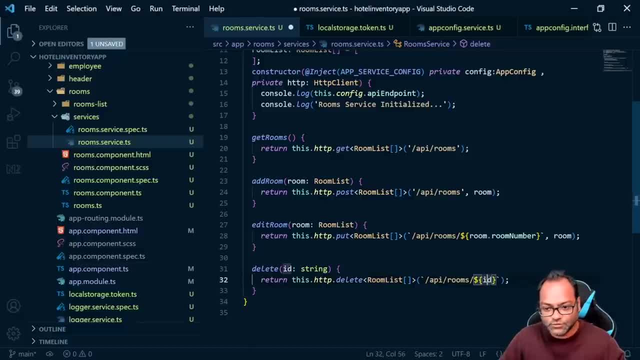 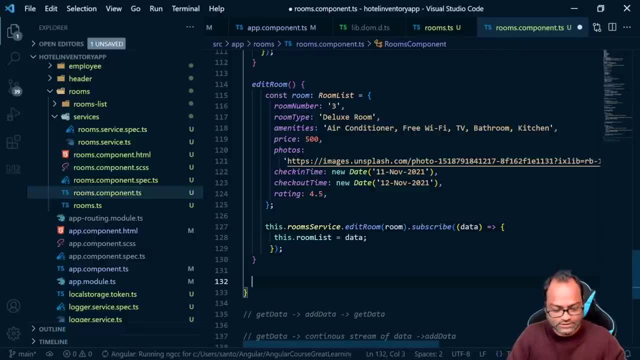 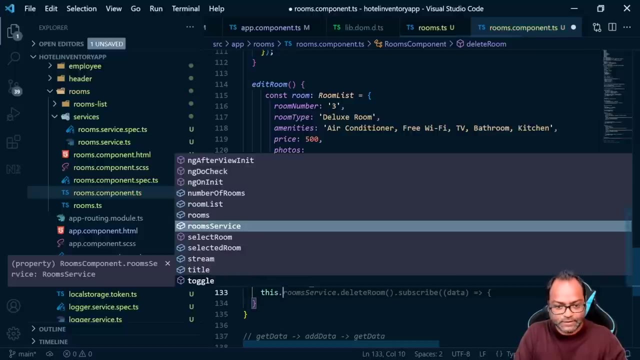 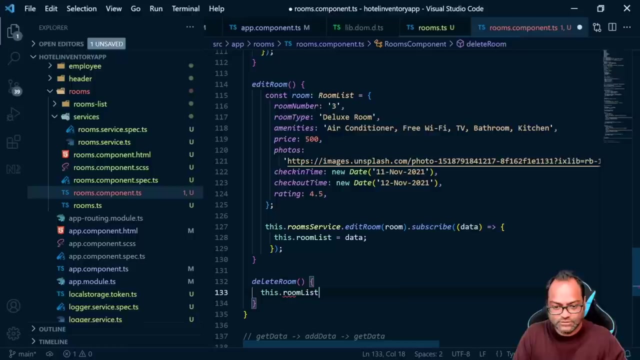 delete will never return anything. that's, that's the, that's true. and let's call, let's say this is delete room. and here we will say this dot, delete room, dot, I'm sorry, this dot your service room service. again, as I said, I'm giving the entire record and let's try to delete this one with room number three. 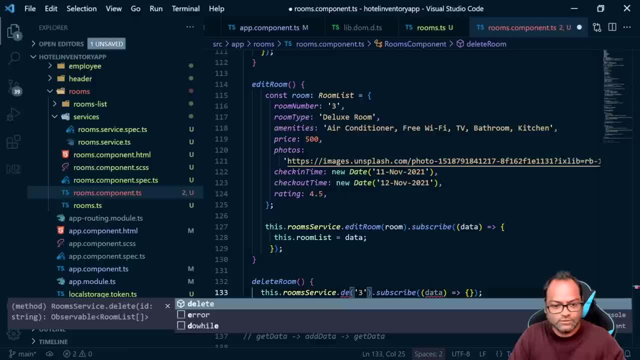 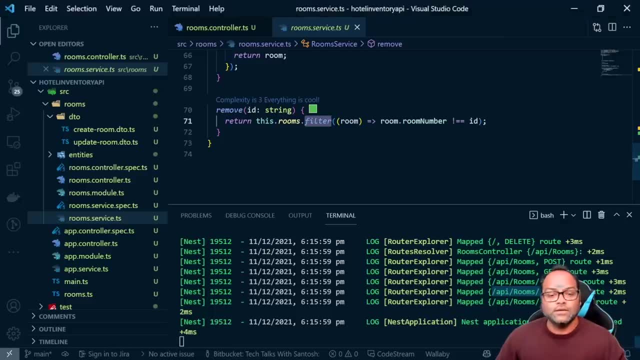 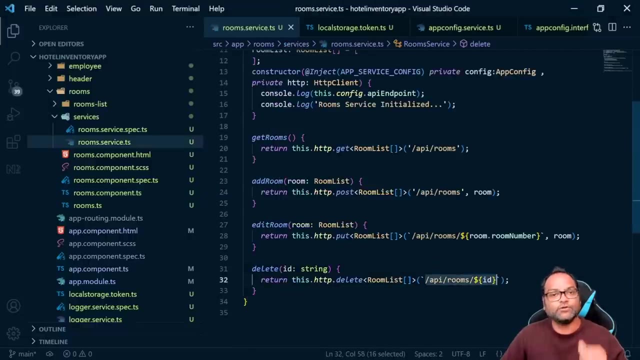 from service: delete, okay, and let's try to assign this data here. so we have- let's see- api slash room slash id. this is how our request looks like right now: api slash room slash id. we don't have to pass any page on this, so we are going to go ahead and 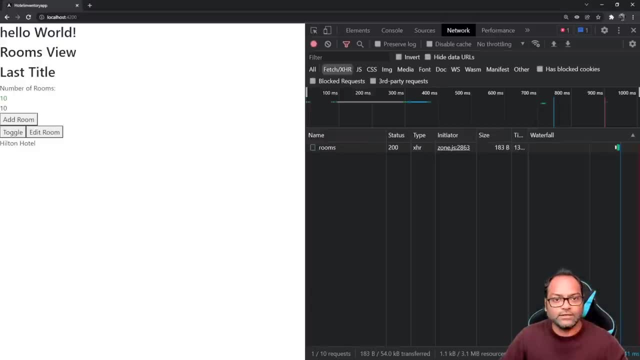 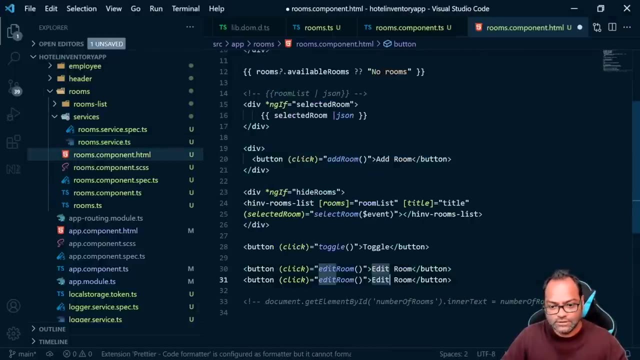 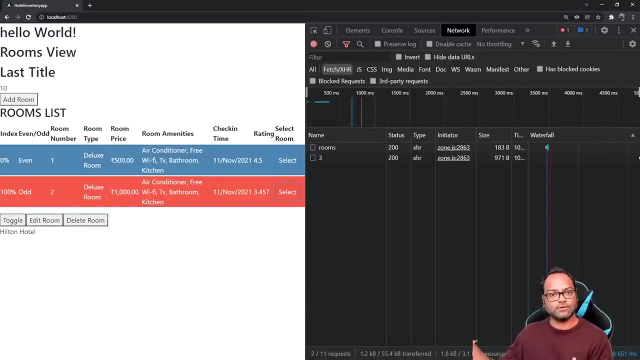 load to delete, go back and we need, of course, and delete from delete button available to call the delete. so i'll say, okay, this is delete room and we will be calling this delete room function from here, and let's go ahead and see the data first and let's click on delete room and done so now. 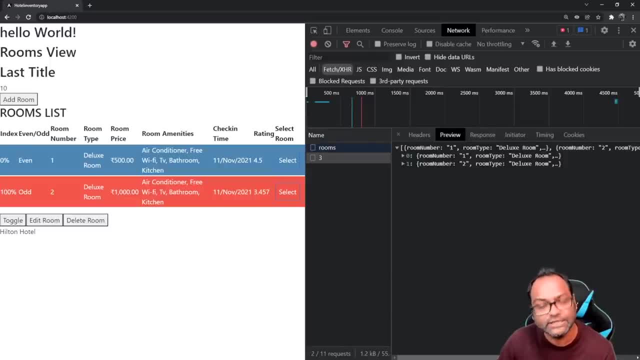 we have learned about the delete function as well. right now you can see it returns something, but in probably in real time, your real time application, it will just give you information about. okay, whether it this data is related or not, or in case you have received some other error, right. 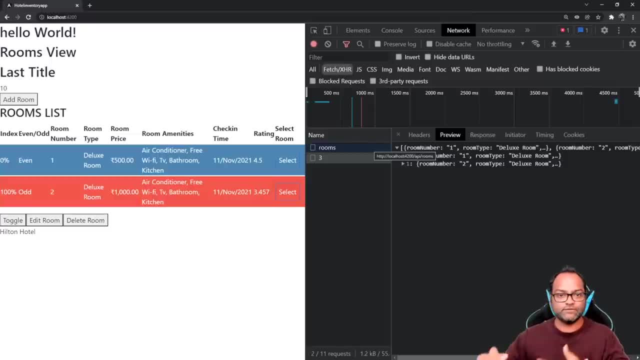 that might, that you might get. but delete generally just performs a single operation. okay, just word and remove this data and that's it. and in case you are also taking care of your apis, make sure you don't delete the data from database. always prefer soft delete over hard delete. so soft delete it means that you have some flag. 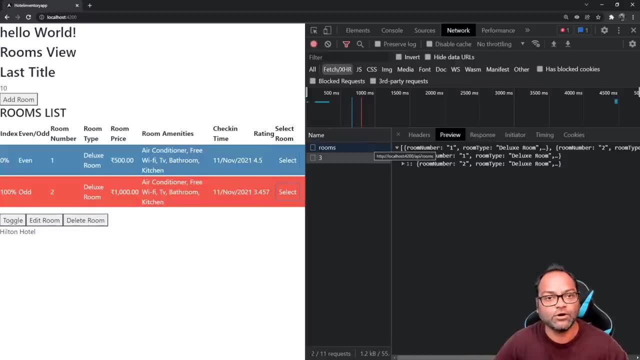 which we just turn on. so probably you can just have a column called deleted and just mark it as yes, deleted, yes, and that's it. so that's it from the crowd operation. you now understand operation. we will see some of the rxjs operators next, and then we will wrap up the http method by 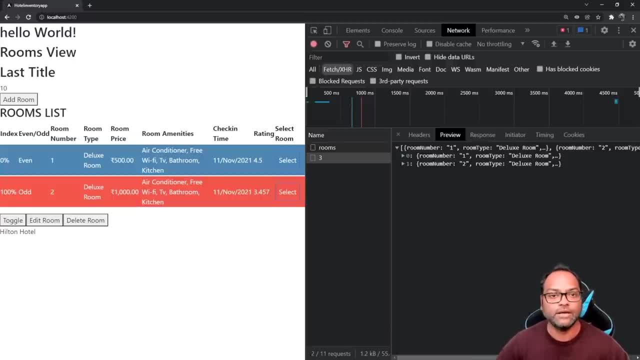 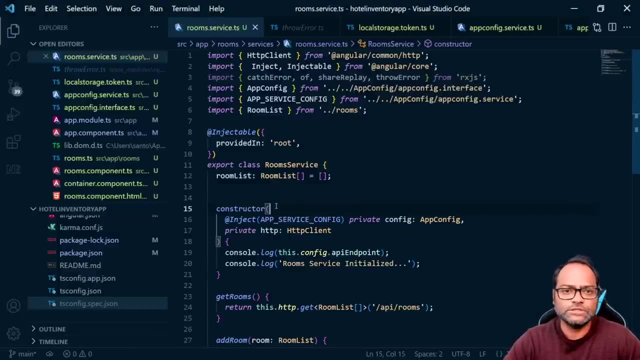 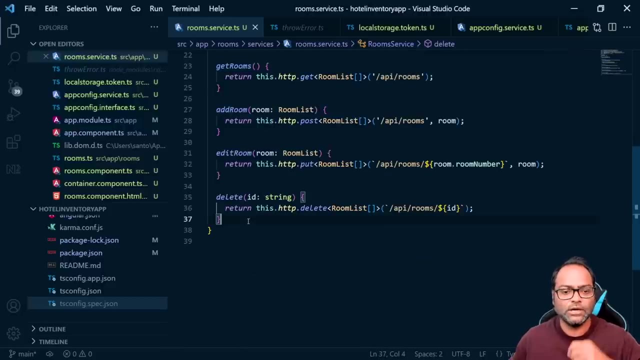 after completing few more videos like app in Next, what we are going to do is we are going to explore one more API which is really powerful. It gives you more information about your HTTP call and it is known as request. So one thing before we go ahead and implement this request API: I need an API which has 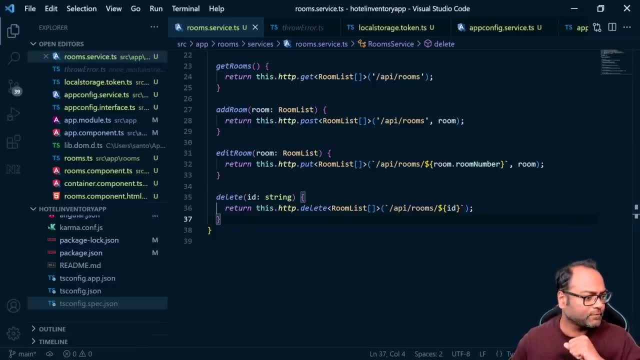 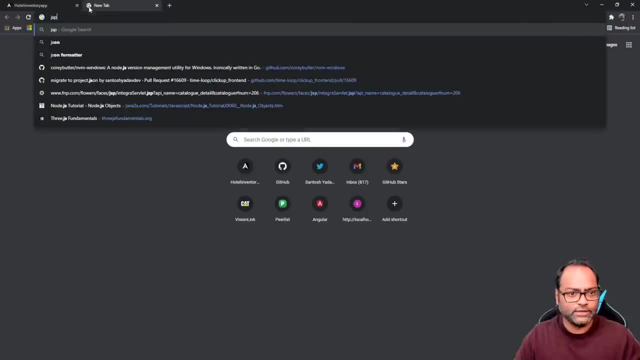 a lot more data. So what we are going to do is we are going to use a dummy API which gives us around more than more than 4,000 records, And JSON placeholder is one of the dummy API, which is which exists. 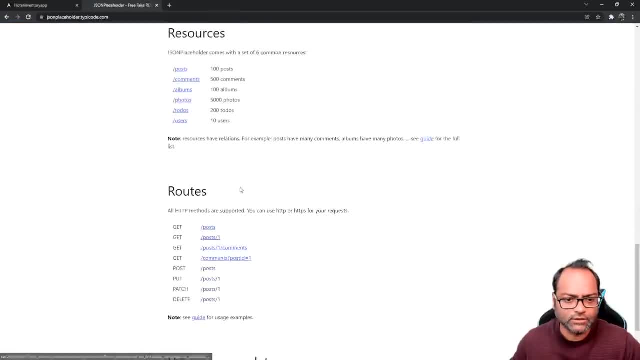 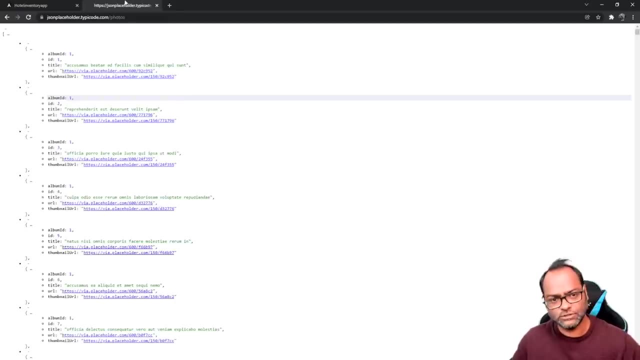 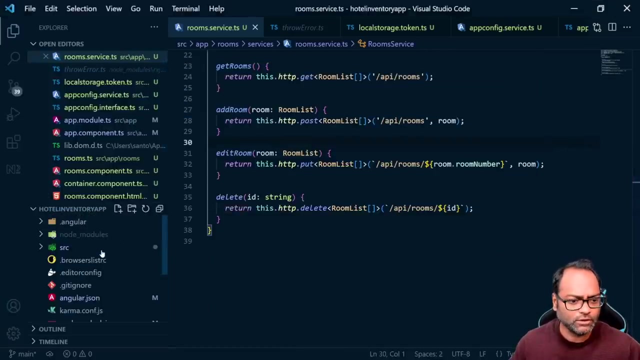 It's a fake REST API and it has a method called photos, which gives us 5,000 records, which will be sufficient, which actually suits the purpose for this particular example. So let's go ahead and do that. before we move into this, I'll just make one more change. 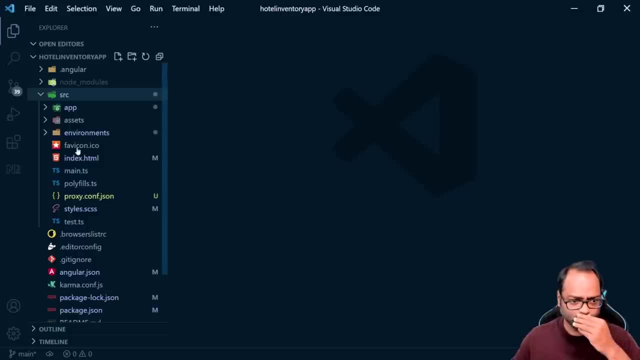 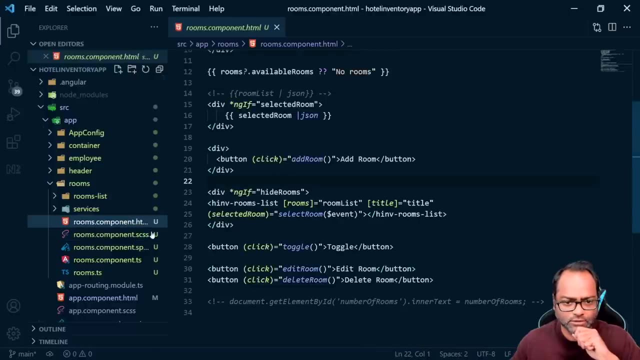 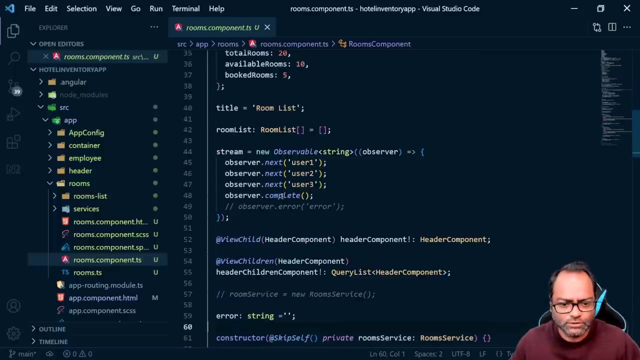 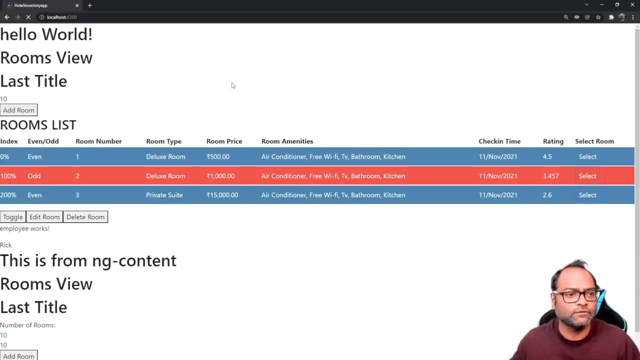 Let me just close, All right, Okay. So let's open the files and in rooms component, I'll just toggle change the value of toggle because right now, by default, the rows are written, which we don't want to. So let's change hide rooms to true, and I think it should work. 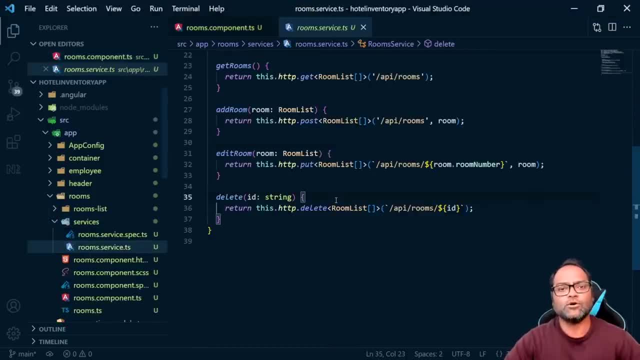 Yep, Let's write this API call as part of REST API, So I'm going to call it room service itself, and I will. we will call it as get photos. This API is known as request, So the first thing which we have to do is we have to go ahead and create a request HTTP. 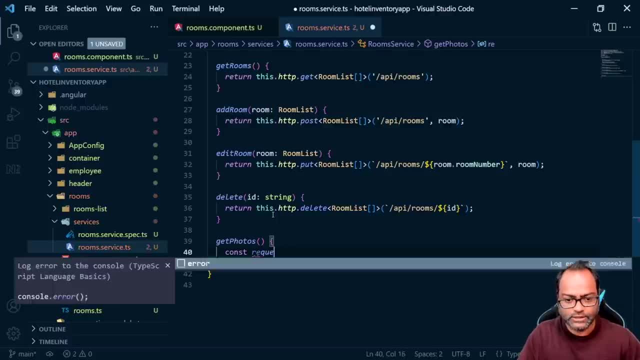 request. So let's go ahead and see how we do that. So I'll create a constant request and is equals to: we'll say this dot- sorry, not this dot. we'll say new HTTP request, Which I'll create, Okay. 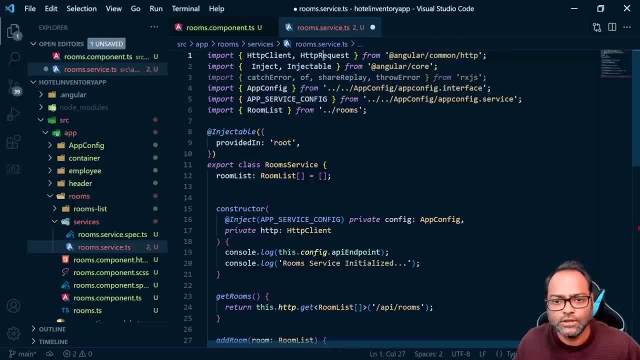 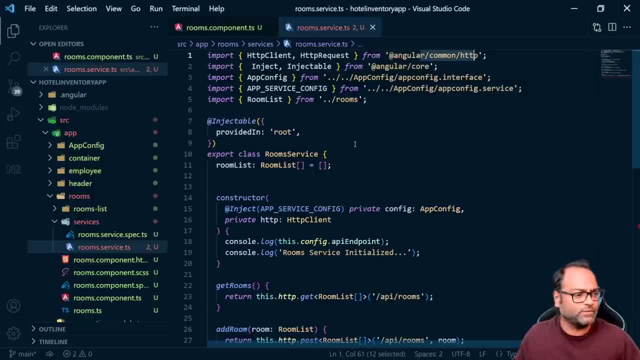 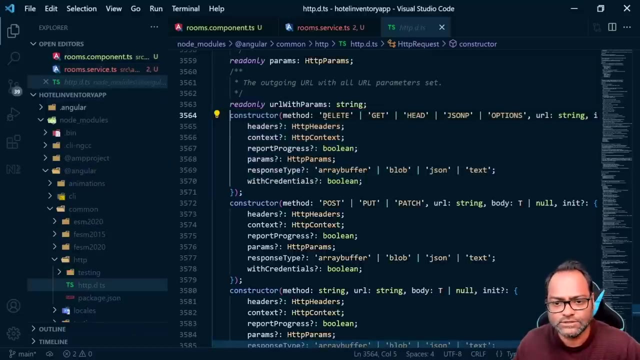 So you can see, actually comes from here, HTTP request which is coming from here. Let me just move this which comes from Angular slash, common slash HTTP, And we are going to. so let's go ahead and see the payload So we can actually pass several methods. 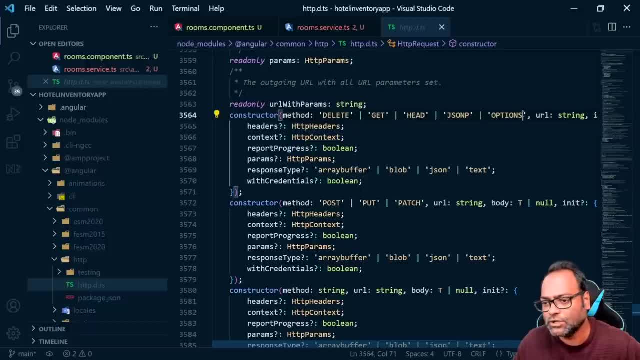 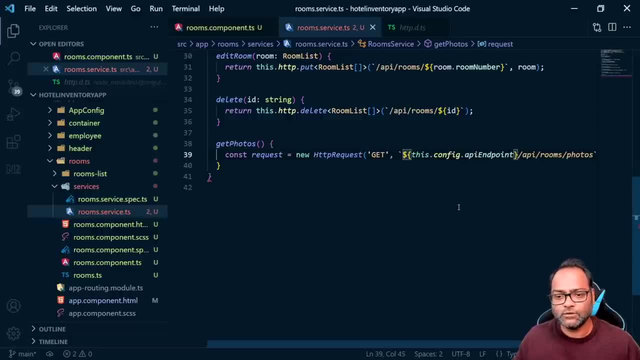 We have get head post. sorry, get head JSONP options, But remember this doesn't work for post because post is not here, Right? So we will be calling get method and this is the API which are which we are going to call. 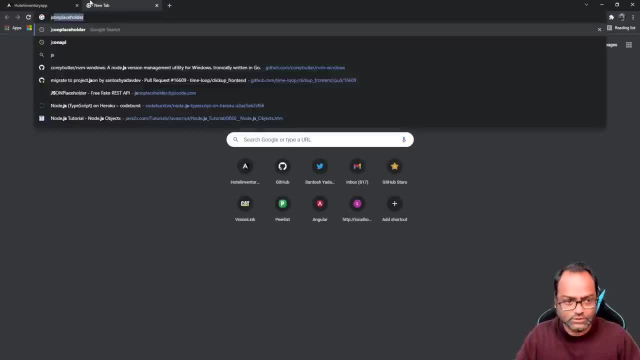 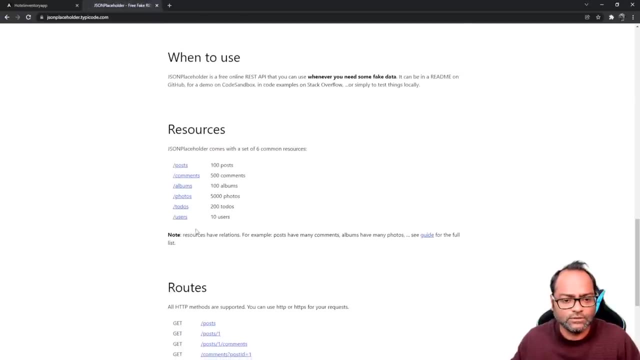 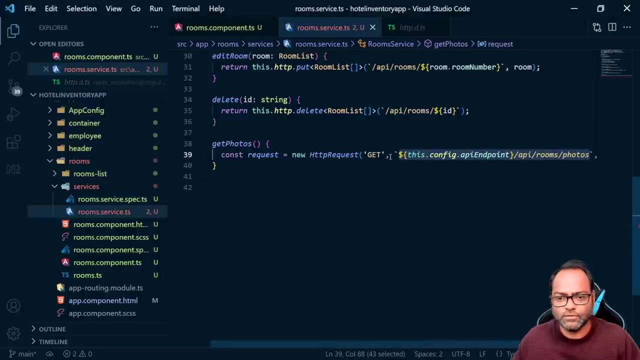 Sorry, Let me just check this in place folder And let me just copy the URL again In case you are trying for yourself. you can also refer this JSON placeholder API for your, your project. So this is the API, And now it needs. 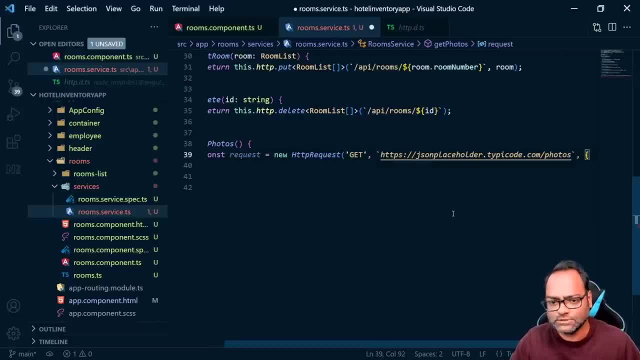 We need to pass some configuration here, So let's go ahead and see what are those configuration. So we are going to use report progress for this particular example that's. And now we are going to pass this HTTP request to our request method. So let's do return this dot HTTP request and we are passing this particular request. 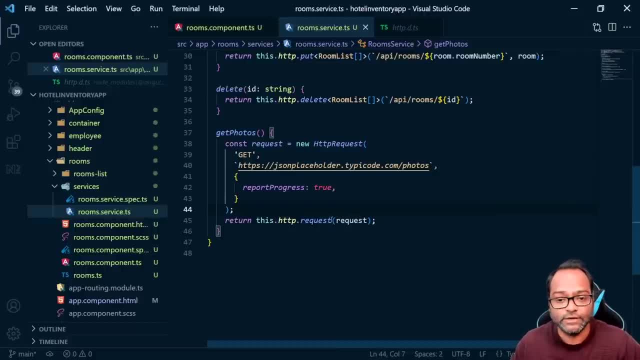 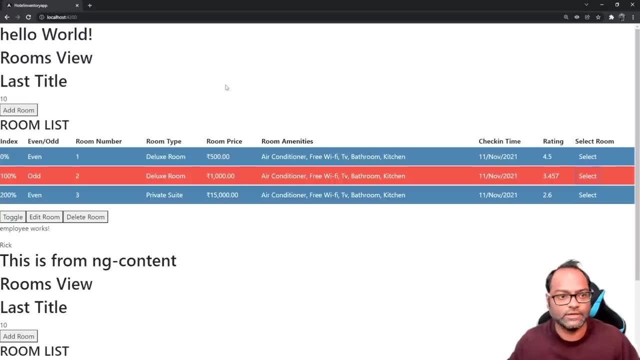 And we need to create The interface as well, because we need to provide the typing. We will do that, but I mean, that's that's for you. You can try this out. You can just refer the metadata or you can refer the properties from this particular. 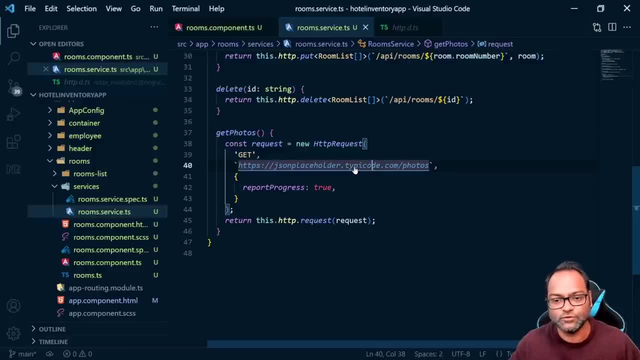 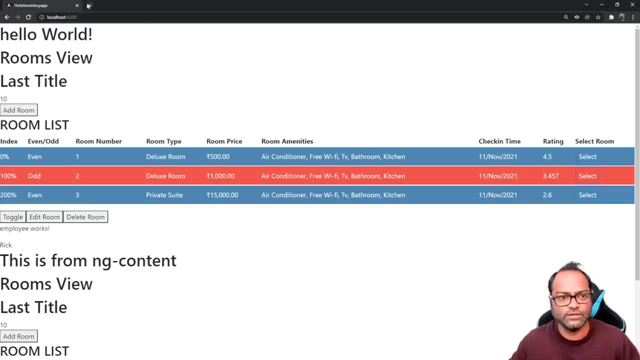 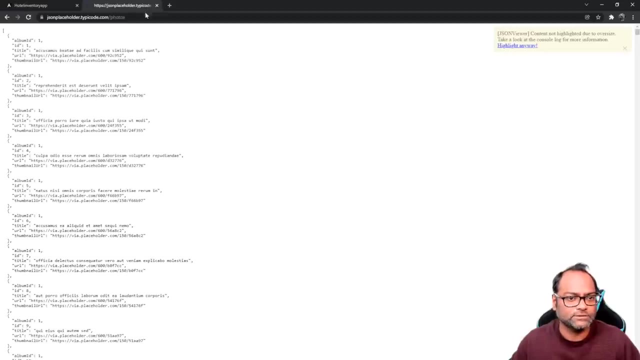 URL, just some placeholder type, code type codecom, slash photos, And it gives you a response. So you know what type of response you have and then you can create your interface based on it. Okay, Okay, Okay, So you have a mighty title. 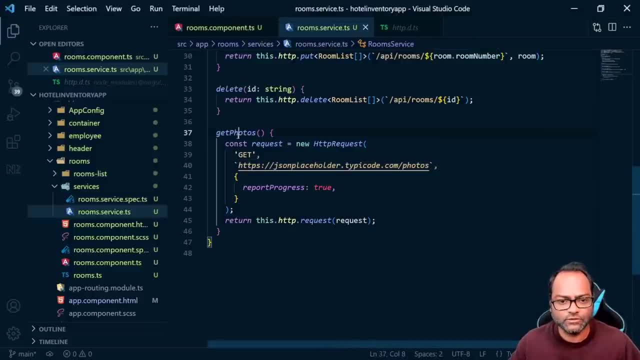 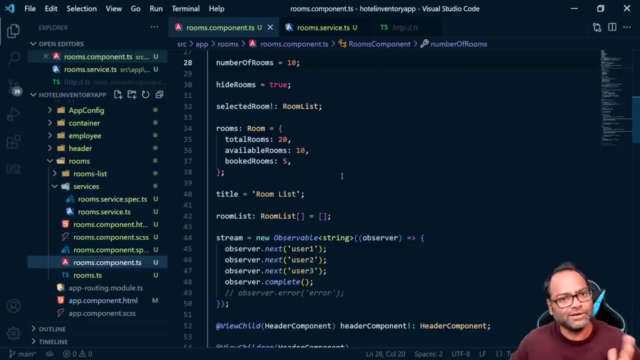 So all of this parameters. Now, once this is done, let's go ahead and call this method inside room component or DS. I'm going to call this method. I'm going to call this method on engineering it. This is just an example, right? 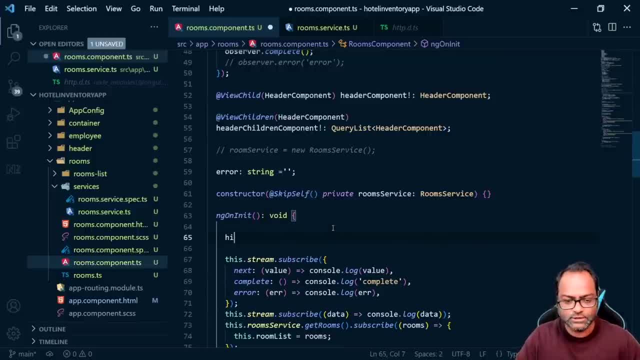 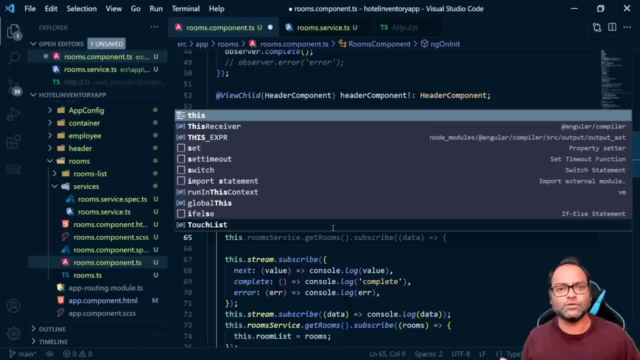 So, in case you need to use this, you can. So let's see what are. as I said, this is going to give you more information about your recipe request, So let's see what those information I'm talking about. So I'll say this. 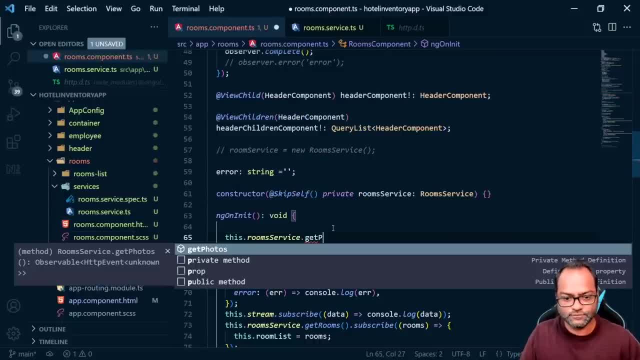 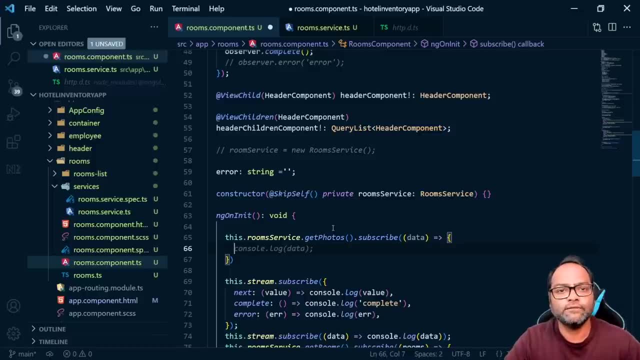 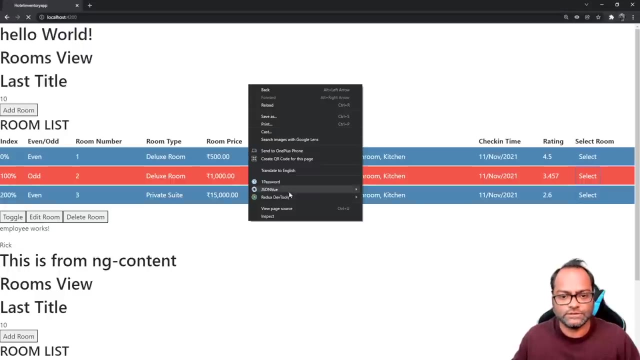 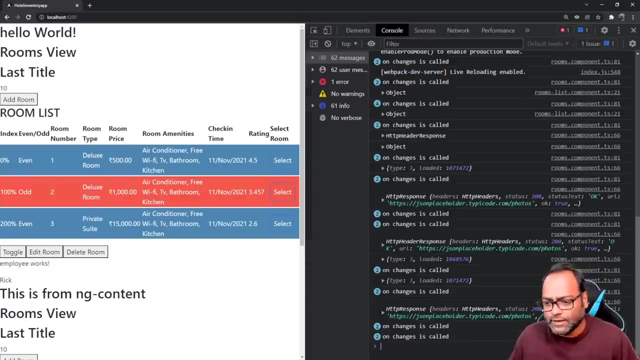 Dot Get photos. And here I'm going to do subscribe and let's see, the first thing which you should always do is just check what the data is or how your data looks like. So let's see. So I'm saying, I'm saying console dot log data and go to console and this room number 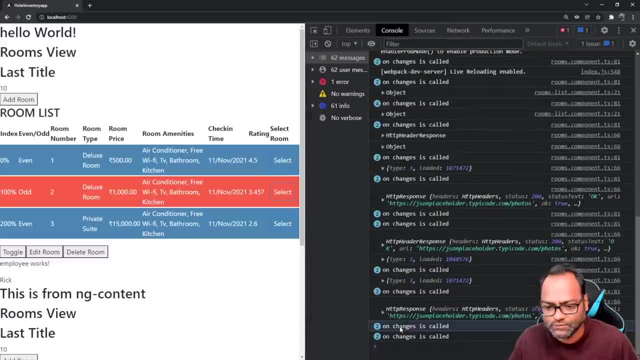 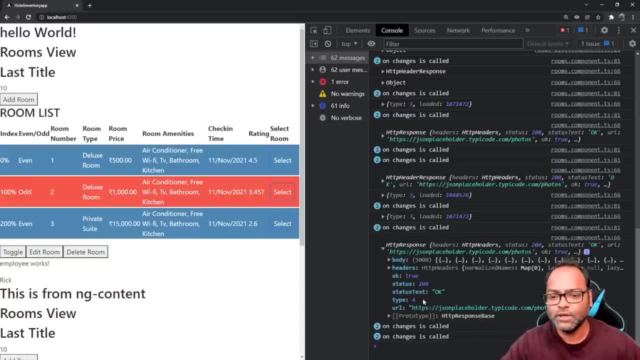 component, or TS line number 66.. And let's see the response. So remember earlier, whenever we subscribed to our data, what we got. we got the data, That's it. But here your rooms component is actually giving you more than this. 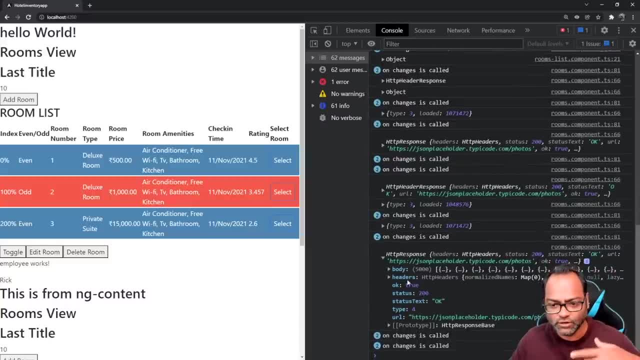 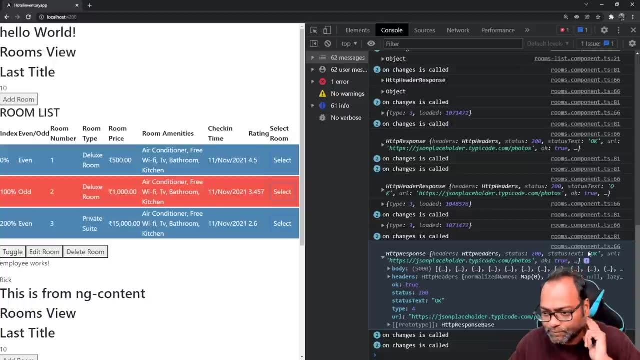 It is giving you entire HTTP response which has a lot of information, which has body status, code status, text. But one more thing: if you notice your HTTP call, which you made using HTTP request and then we subscribe to it, it is actually printed multiple times. 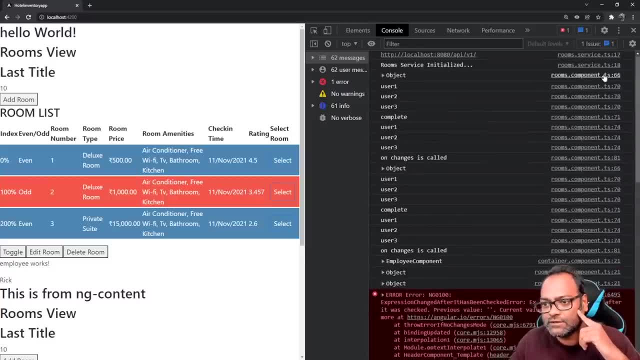 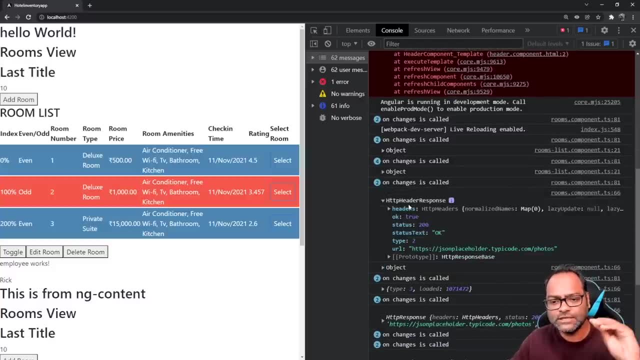 So let me just start from the top right. So here we don't have anything, but we have to see for line number 66. So here. so first is here, So you can see it has some information. It says: HTTP header response. 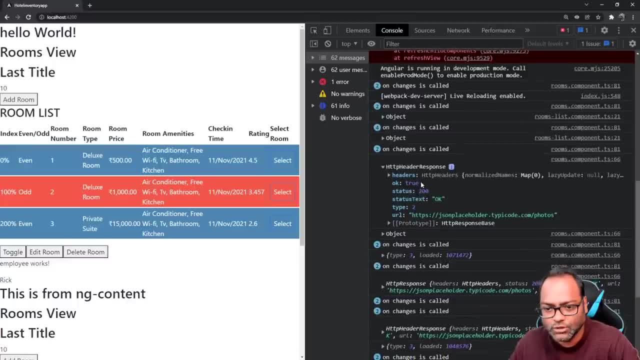 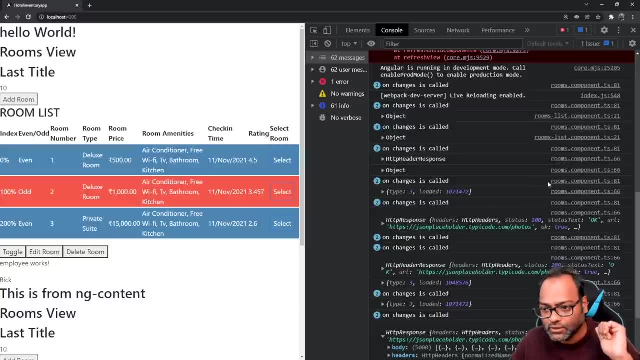 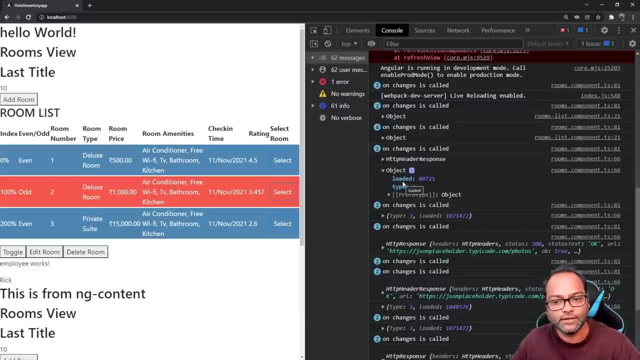 So it says, okay, uh, your request to the server is sent. This is what we get. This is what information we get here. Okay, Okay, And now this is also 66, and here it starts loading the data. Okay. 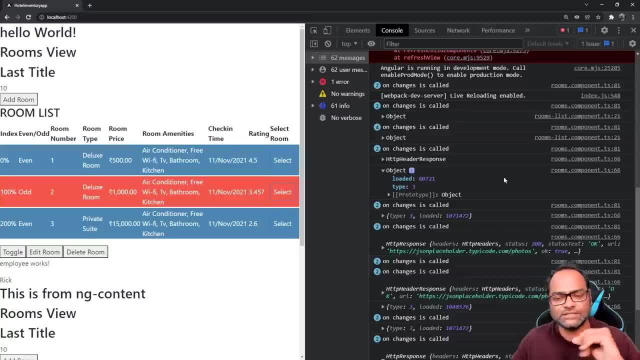 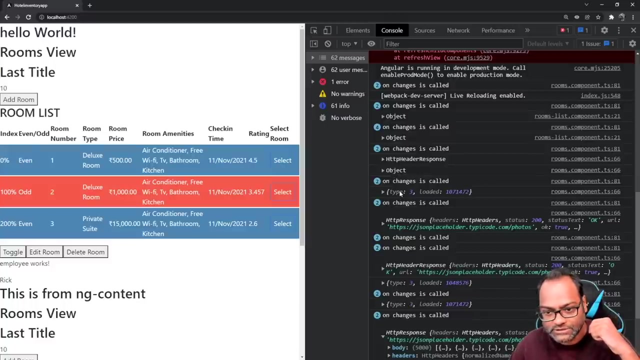 So here you can see at this line again, this is line number 66. So this is where it actually start Start loading the data. So it also gives, So it also gives you information how much data is loaded. So you can see here line number 66, again line number 66, here same 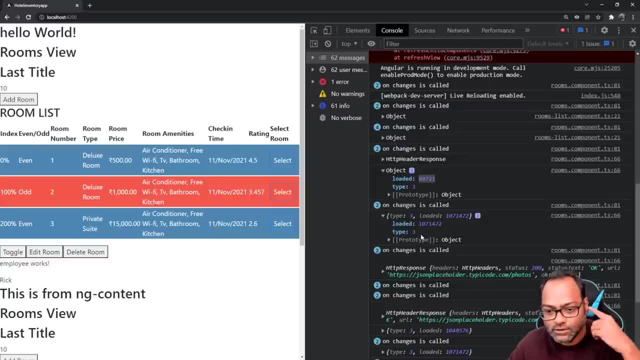 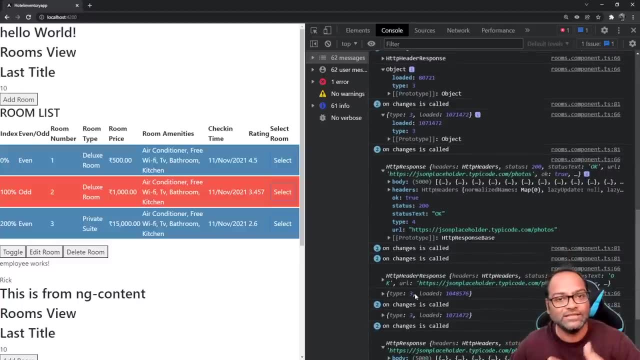 If you see object type three and how many bytes are loaded here again, and then finally, when you get the data, It gives you the data. Okay, It gives you HTTP response. Why this is printed twice? because we are loading it twice, right? 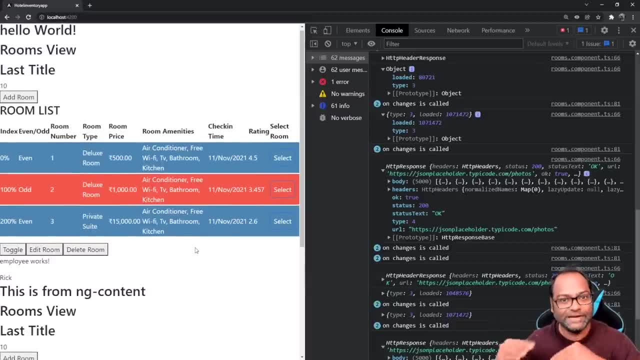 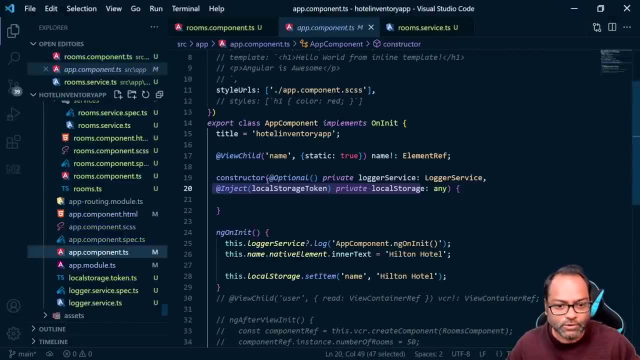 So you can see here it's the same component, a room component, getting called twice, So you can you get same information again and again. let's hide one, So I can. we can go to app component dot HTML and side this: 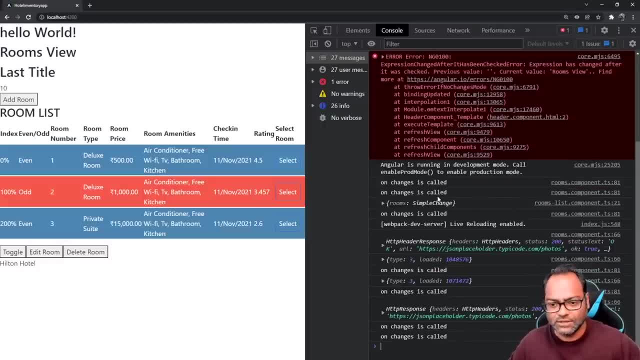 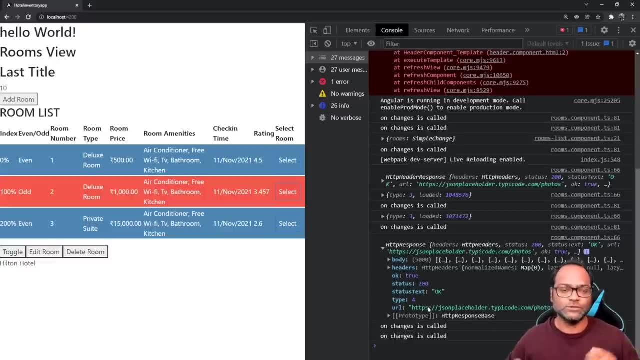 And we will. so we will see get some. sorry, we'll get small log to work with And yeah. So now at the end we have this HTTP response- What you can achieve using this. So let's say, if you have any API which takes some time to load data and you have a lot. 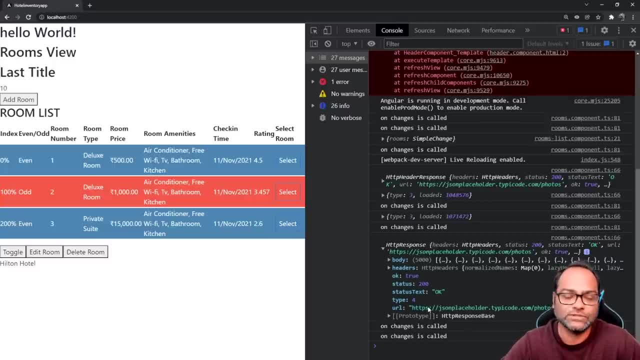 of records to display, for example, the same example. right, We have 5,000 records, So we don't want to actually Make made us, we don't want to you make user thing that this is, the application is and right now, but rather you can display the user that okay, this many invites are downloaded. 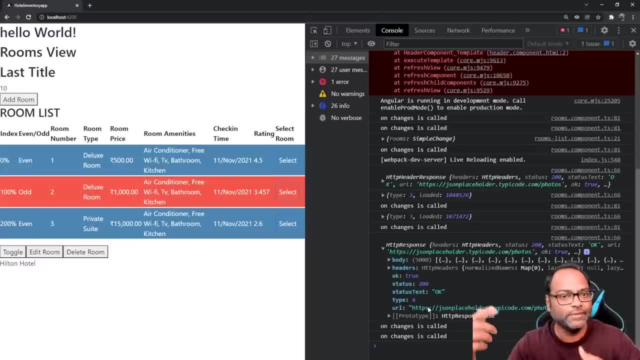 and you can probably show some loader, right, Yeah, And based on that, your user- I mean even your application- will be interactive rather than actually just being there, and user thinks that, okay, there is nothing which is happening. So let's see how we can read this information. 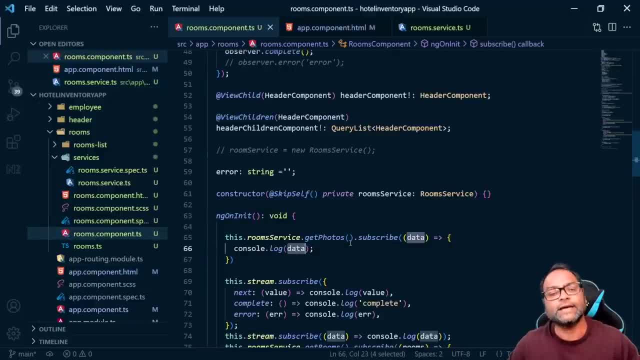 Let's go to room componentts. So this data is actually not the data, It's event. So if you see, there are multiple events which is being called, So I'll call this as event And then here what we can do is we can subscribe to multiple events. 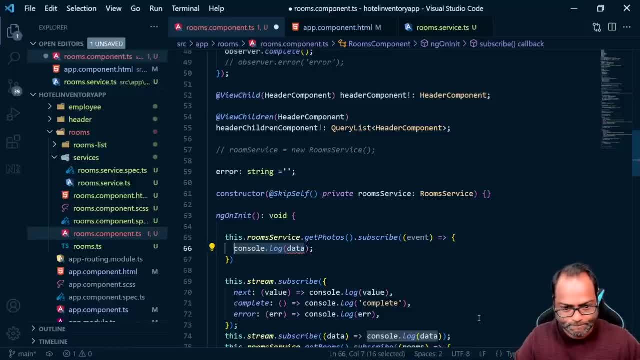 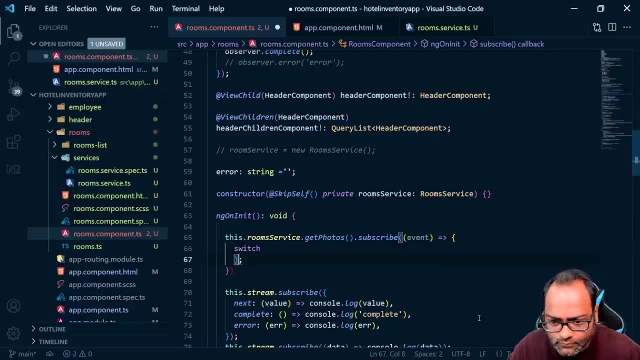 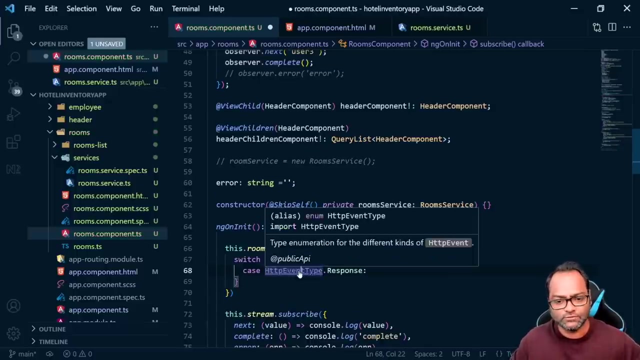 So I'll say, okay, let's use switch. Okay, looks like some. okay Switch based on the event type. I'll say, In this case, first let's see HTTP event type, which we have to import. HTTP event type is what is going to give you those information. 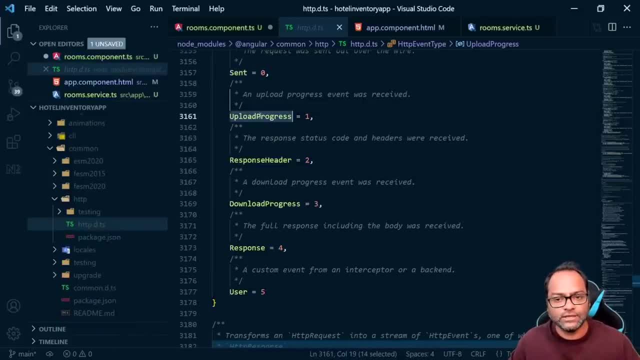 So, whether your request is sent, I mean in case it's an upload event, if upload is in progress, if it is download, what is the response header? whether our request is actually sent to the server or not, in case there is some problem communicating with server you. 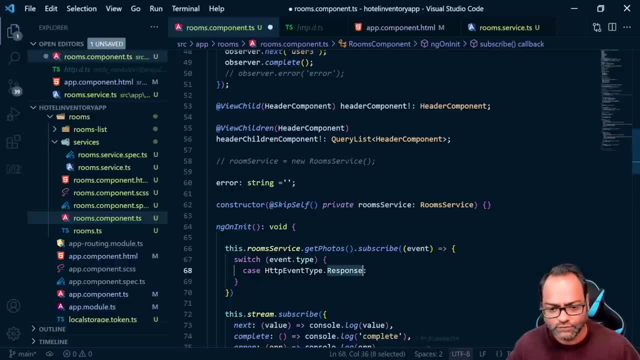 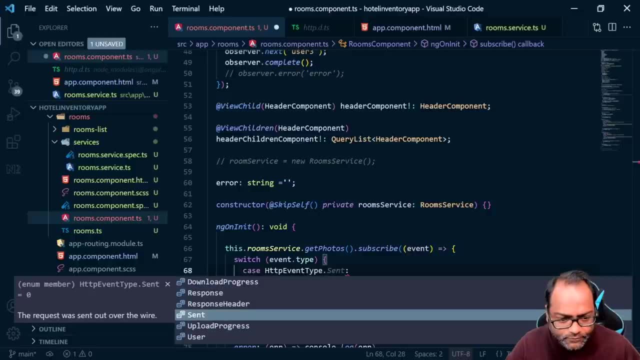 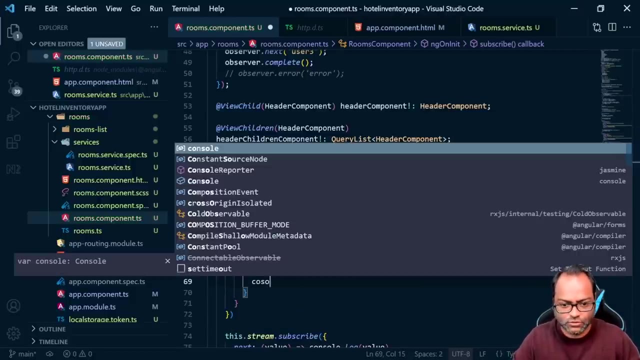 will get an error here And let's go ahead And do that So first and we are going to see, we are going to say okay. So, in case the request is sent, and say okay, console dot. log. request has been made. 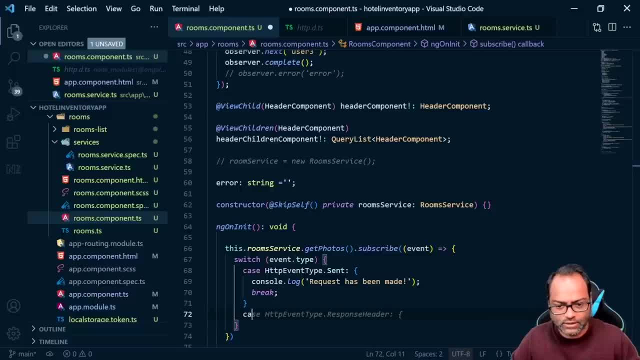 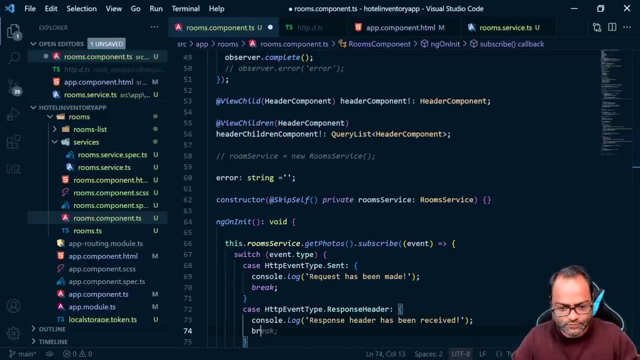 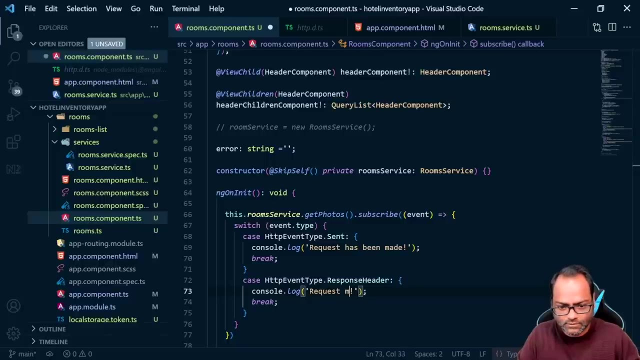 And of course don't miss the break. Then, case, I'll say this is HTTP response header and say console: Uh, and Here we are going to say request success. and then case: this is uh important. So we are saying: okay, case, HTTP event download progress. 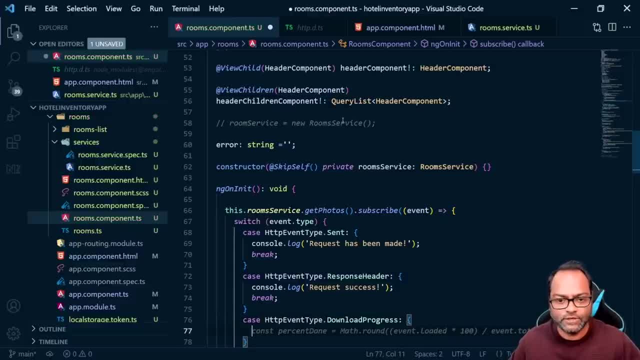 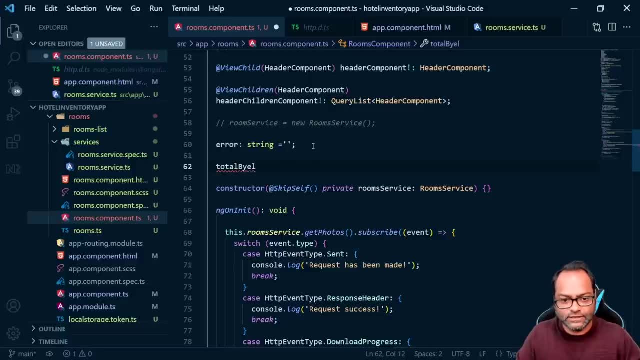 And here what you can read is: uh, let's create a variable. I'll say: this is console. Uh sorry, Uh, total bytes. So this event I Is actually going to give us how many bytes are downloaded. 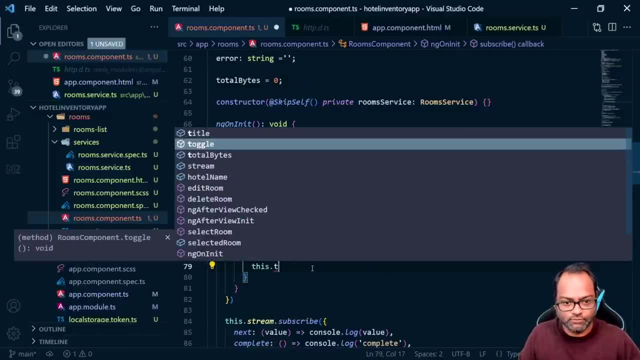 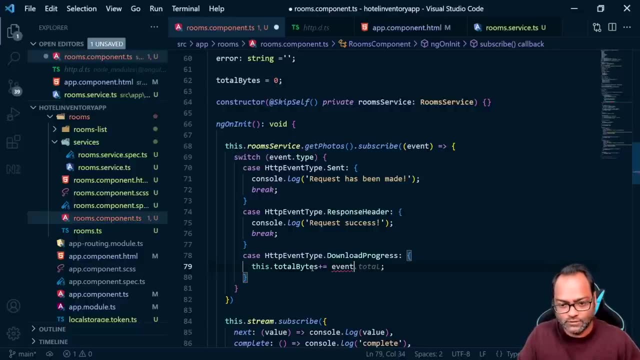 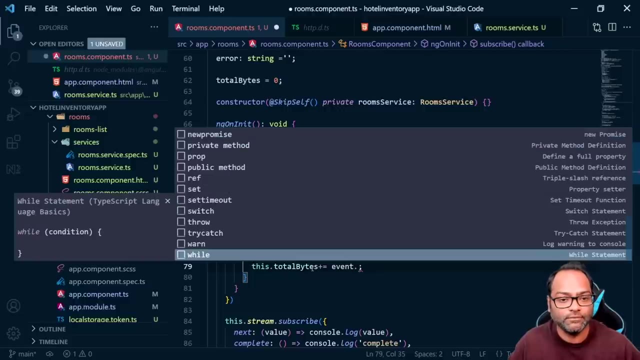 So what we can achieve here is we can say this: dot total bytes, uh plus is equals to event, And if you try to access right now, you will get two properties: total and type. So total can be uh, um sorry, total can be null while you are downloading the data. 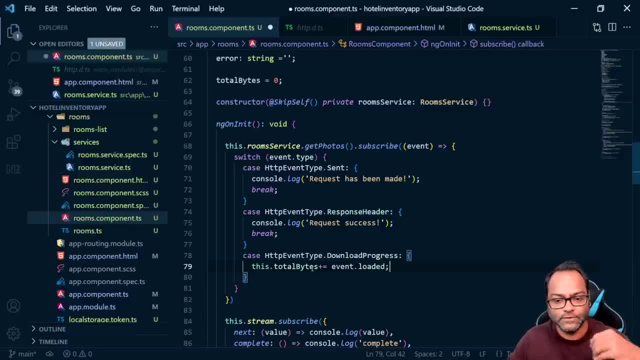 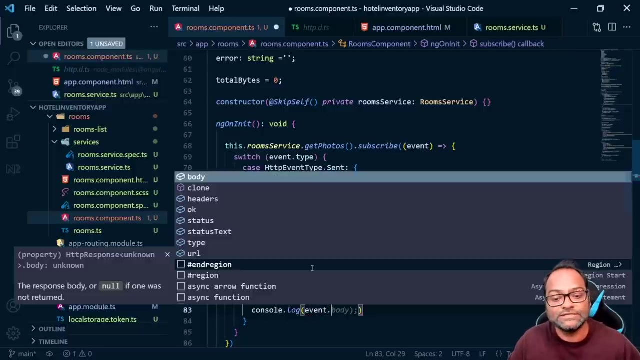 So what we need is loaded, So we need to Show how much data is loaded, and that's about this. And finally, we will handle the response. And now, if I do console dot log and let's do console dot log again, So if we try to access event dot, you will see, you will get uh many properties, and these are the properties which we generally get from an API. 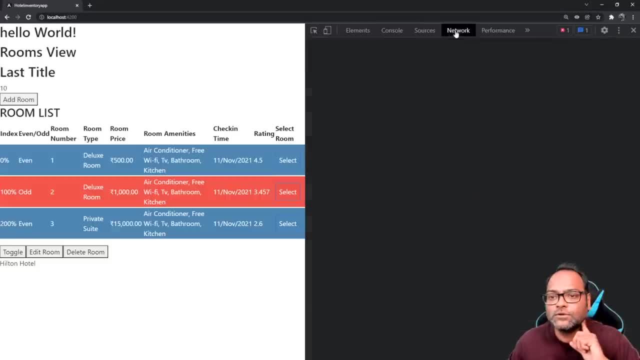 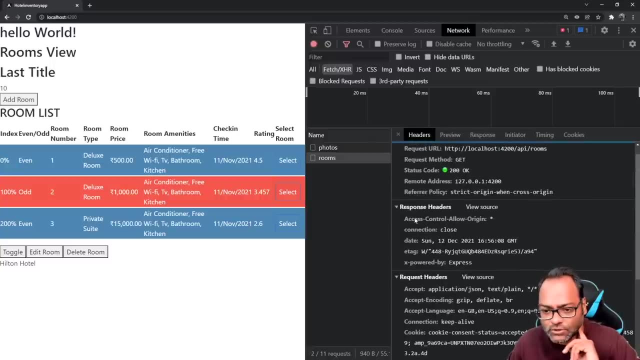 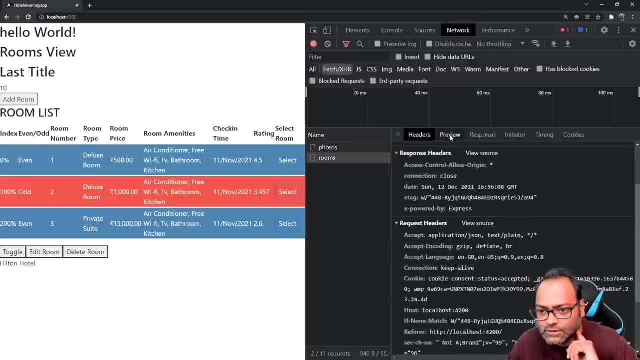 Let me show you. So, if you go to network and click on rooms, click on headers, and you have requested us, right? So sorry, not requested us, but yeah, this one, So you see, uh, you get status code, you uh get the data, of course, which is part of your, uh, your response. 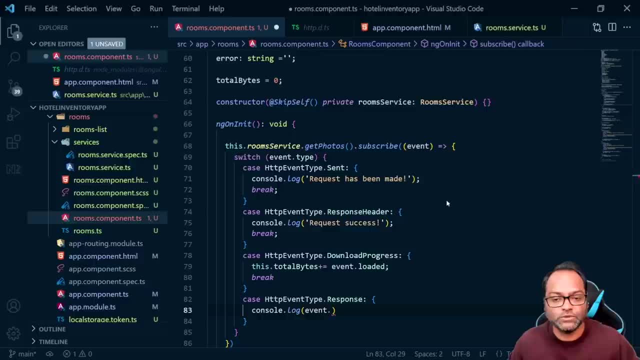 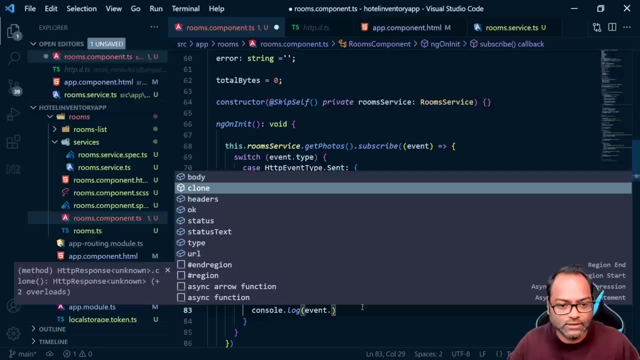 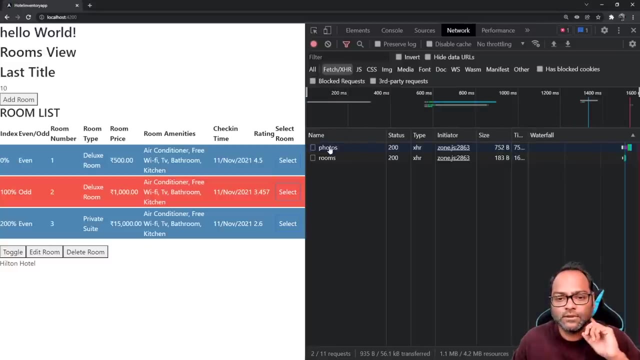 So you are going to get more information about what your response was, including the status board, including your body, including your headers, status, everything. So I'll say, let's try to access body and let's see, and this is your photos. but this is not what we are interested into. 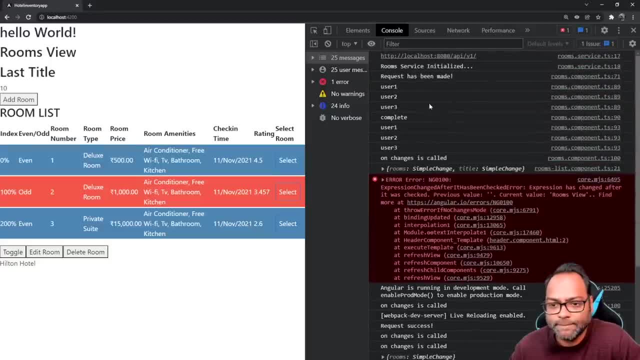 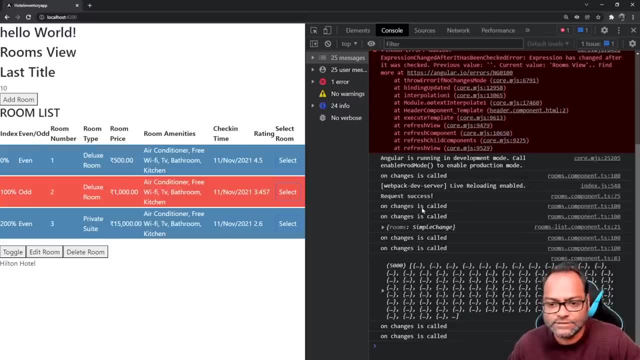 We are interested in console dot log right now, So let's go ahead and see. So we have, of course, this is, uh, this is our data. So this is 5,000 reports which is available And here, uh, we want to display the total. 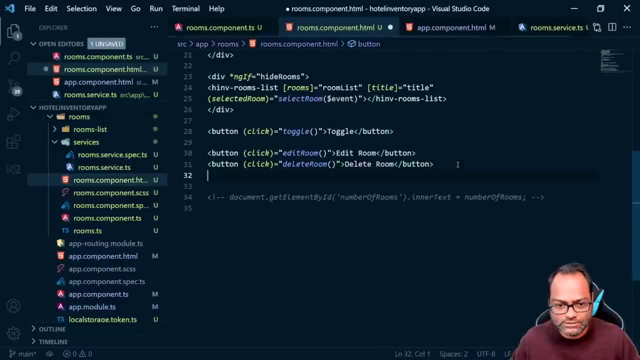 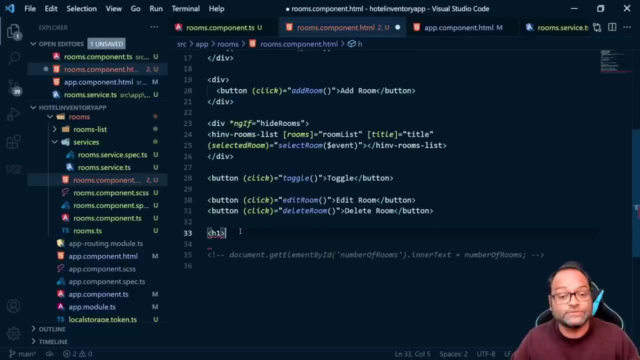 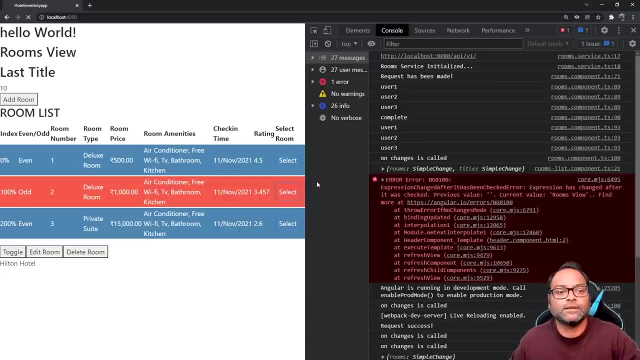 By it. So what I'm going to do is here I'll say: there is, let's play, send H1 here, Sorry, So it is visible. And then I'll say: this is total bites loaded, Let's see, And you can see. uh, of course it is. my internet speed is real fast. 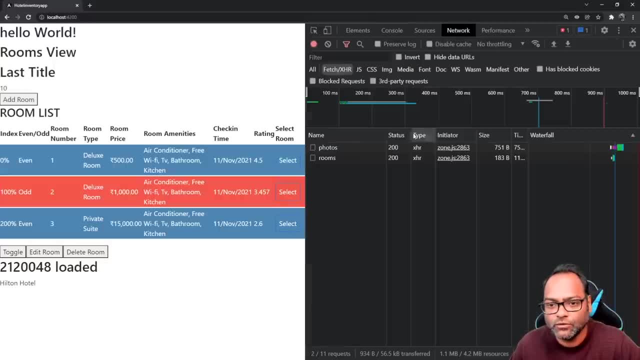 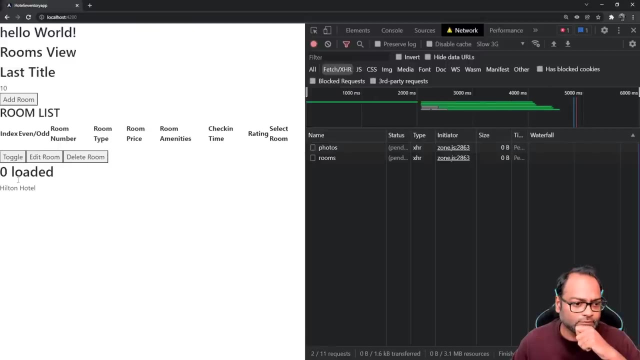 So you can see too, this many bites loaded. but we can go to network and, uh, we can move to slow 3g and let's reload Right. So you can see, okay, it was, it was it started from zero, and then it is loading the data. 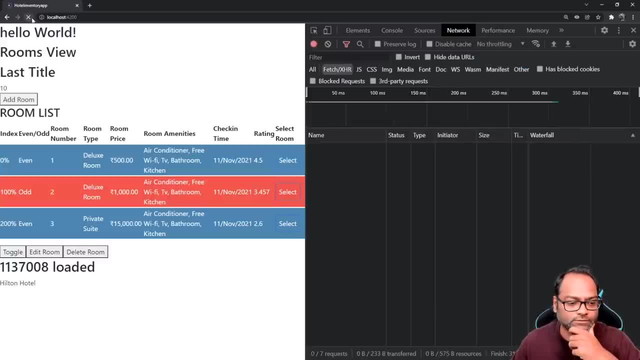 So I'll just go to no throttling again. And so it is too fast, of course, So to download this many 72 bites, So it didn't took a lot of time, But yeah, this is what you can achieve using request API. 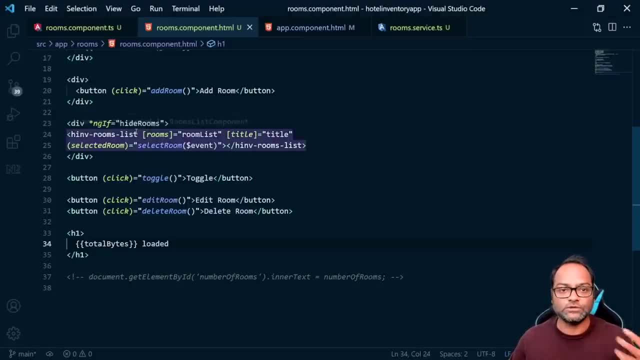 It is really powerful. It gives you a lot of information, more information than what you're you generally get from your certificate, Uh, so try to utilize this as much as possible. We already saw the use case where you can do that. 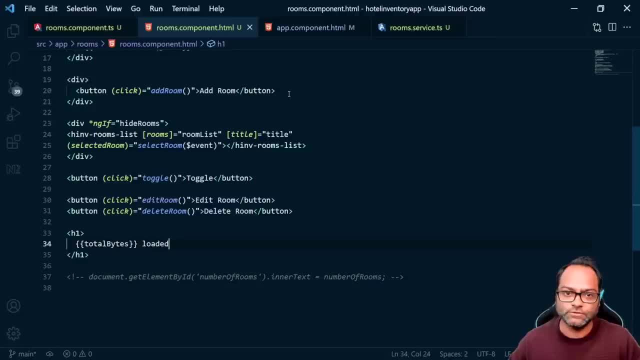 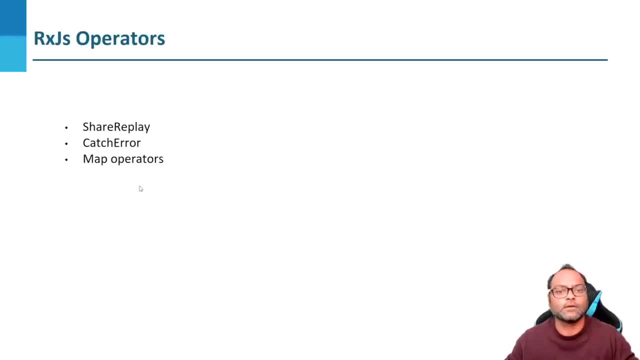 The only thing is we had to utilize the Jason placeholder API because we don't have an existing API which gives us the those many records. So, yeah, that's it. from the Next, we are going to discuss and see some RxJS software. 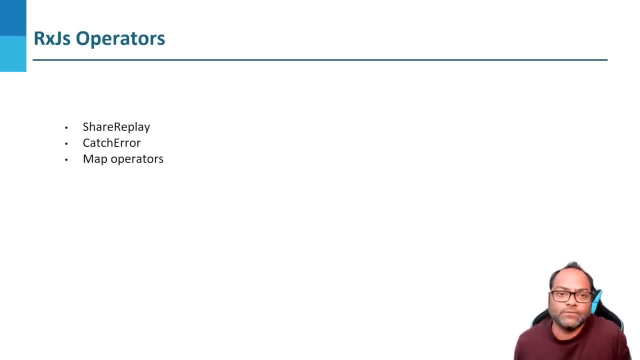 And once we show that to you, that we are going to talk about How to use RxJS, So we're going to talk about the best and the best RxJS software in the market. Uh, today I am going to talk about RxJS as a full-scale standard. 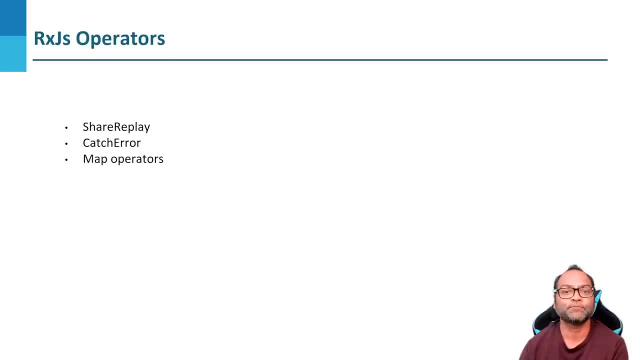 software to run RxJS, And we are going to talk about RxJS softwares- vfx- that I mentioned in the introduction. So those are the two things that we're going to talk about today. So let's begin with a brief introduction. 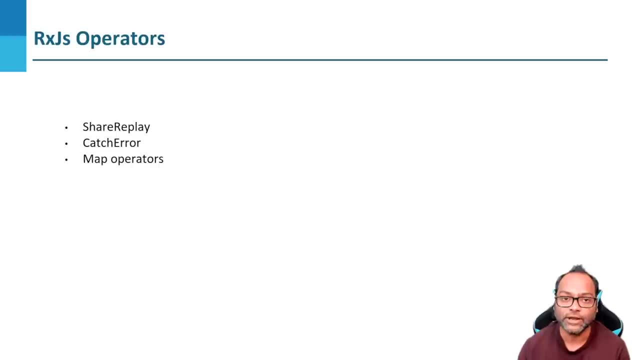 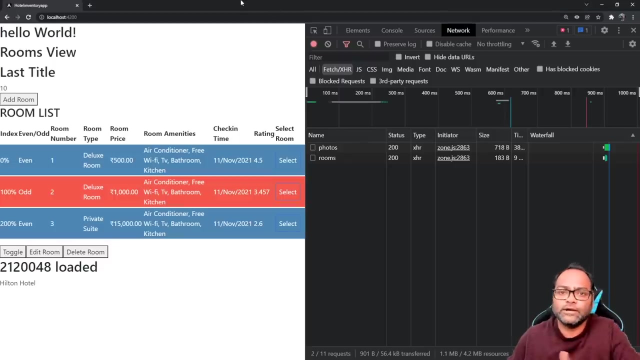 We are going to talk about RxJS code. I'm going to use this. you will be able to use enough rxjs operators as well as well as enough rxjs in your application. there are many operators which exist. there are, i think, around. there are more than 100 operators. 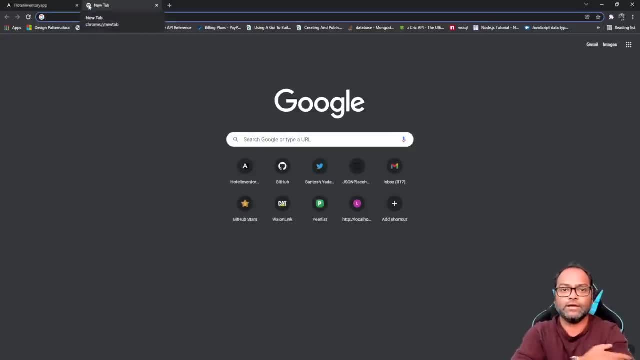 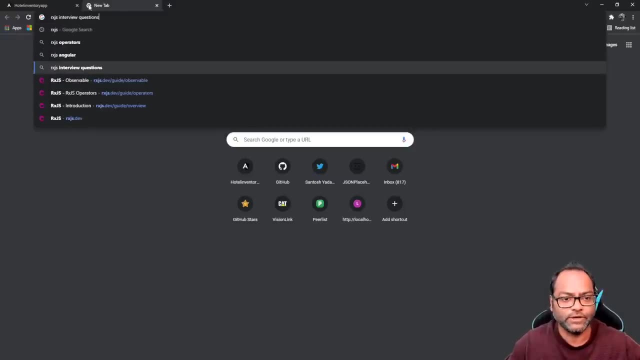 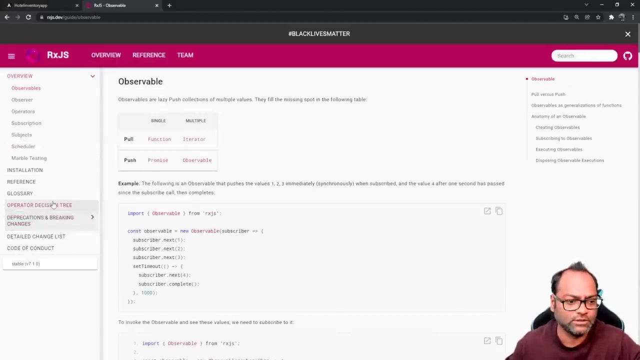 which exist. it's not possible to know all of them, and you even don't need all of them to. to be frank, you can always refer the rxjs operators on rxjsdev, which is official website, and in case you are not sure which operator to use, they have a really nice operator decision tree. 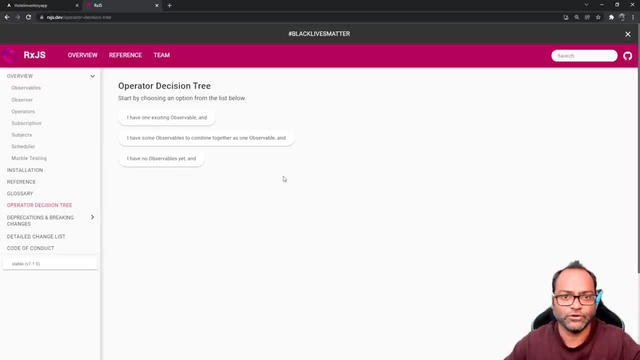 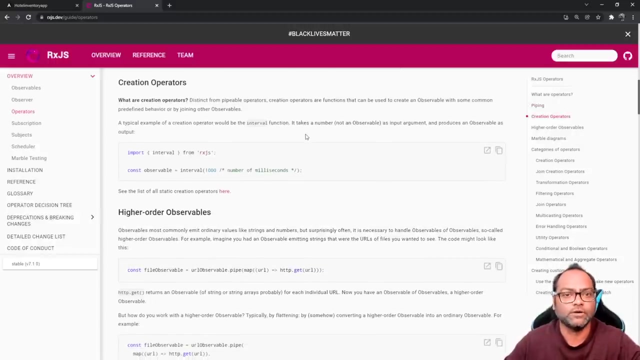 where you can give some information about what you're trying to achieve and they will give you an operator which we can use. you can see the documentation for operators here. as i said, there are more than 100. it's not possible to understand all of them and probably you won't be using or you never need more all. 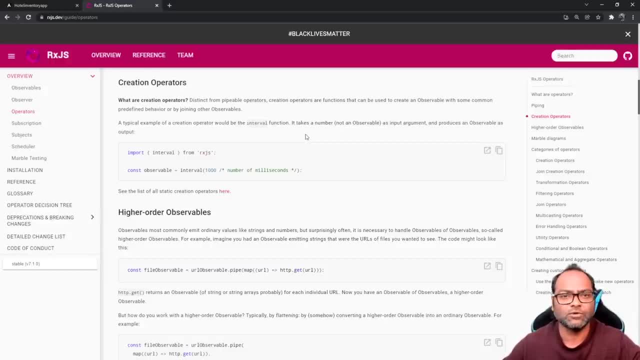 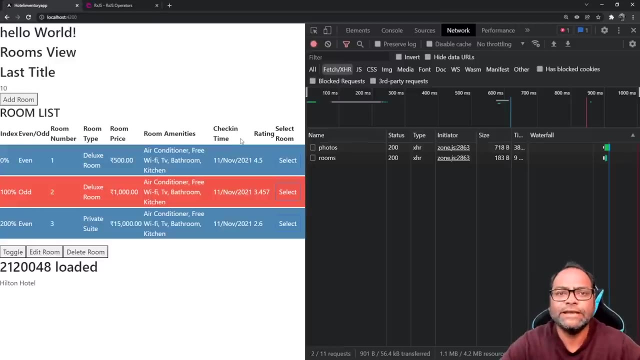 those hundred operators you You're going to almost use, most of the time, around 10 operators, from which we will be covering most of them here. The first operator which we are going to use is share replay. Now why we need RxJS operators. Remember, RxJS gives you a stream of data and that stream of data cannot be modified. 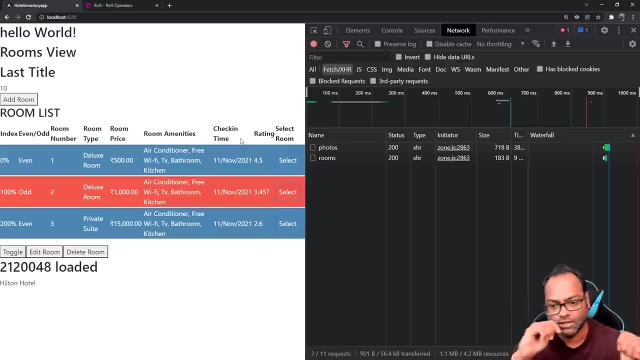 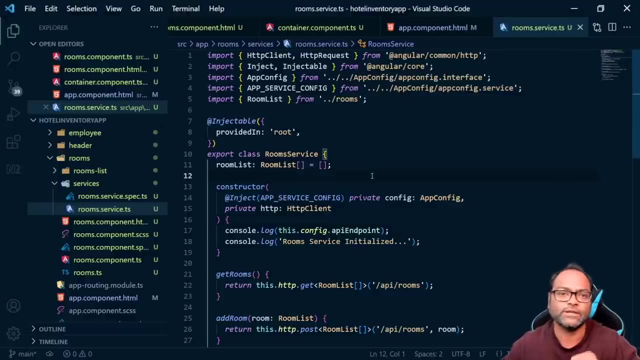 It can be modified only within a stream or before it is subscribed. So how to modify those data? So that's where operators come really handy. So here I'll give you an example of how we can use share replay operator, and then we will also see some examples of operator where you can modify the data while the stream within. 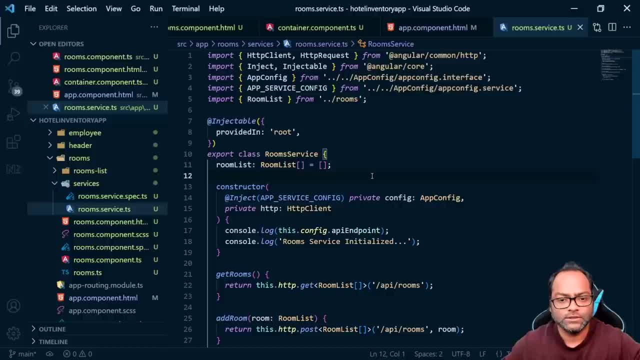 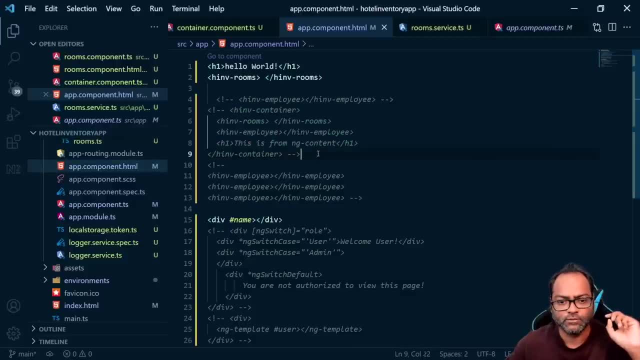 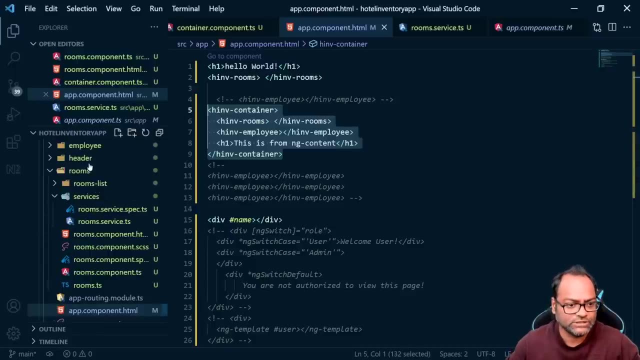 the stream and then give it back To see this example. what I'm going to do is I'm going to make two changes Here. I'm going to uncomment this again, So we get the request twice. I have made one more change in container component. 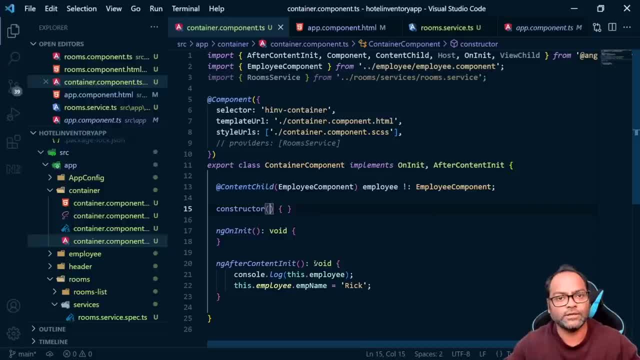 Remember, we had this host decorator here on the service and this. providers have commented this and I have removed this as well, Just to make sure that you are following the same, because if I don't remove it, I mean we are going to end up with multiple changes. 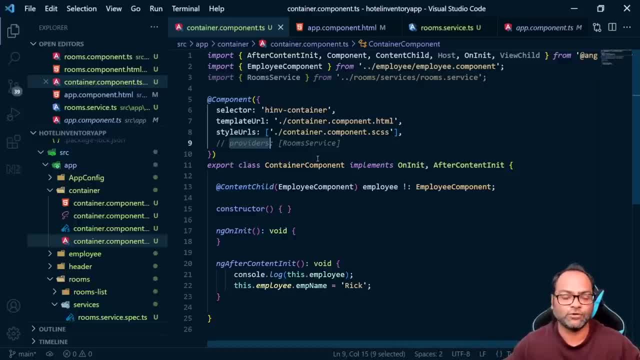 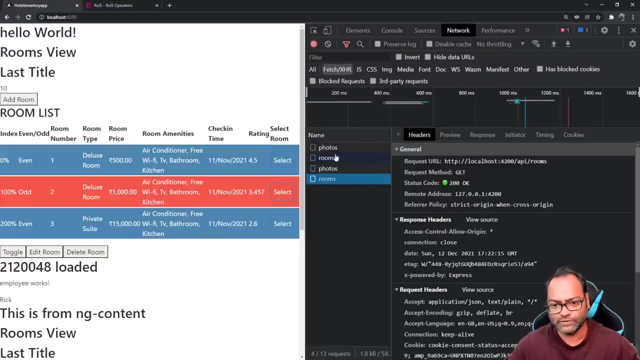 So what I'm going to do is I'm going to make two changes and then I'm going to make two changes, So let's go ahead and talk about this share replay service. So here you can see: rooms is being called twice, Photos is again being called twice. 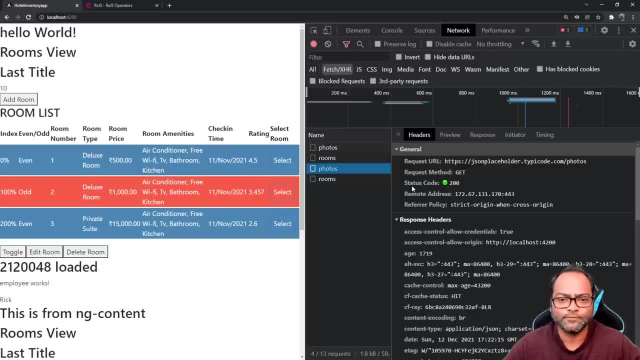 It's the same data, right. So why we need to make two calls? What we can do, what we can do better here, probably we can cache whenever first call is made and then we don't have to make another call, right. 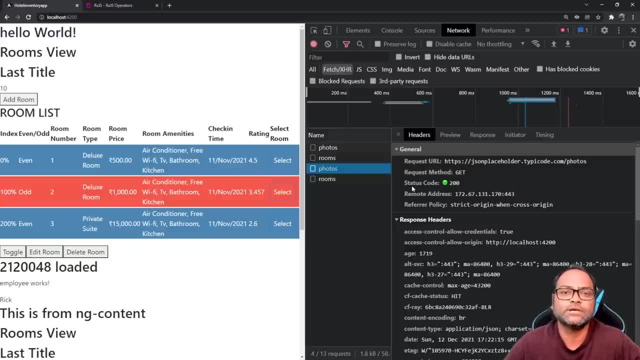 That's looked like a perfect solution. Yes, That's what share replay does. Share replay can help you to cache the request, so you don't have to make your call again. It's very useful in case you have some master data which you don't need to download again. 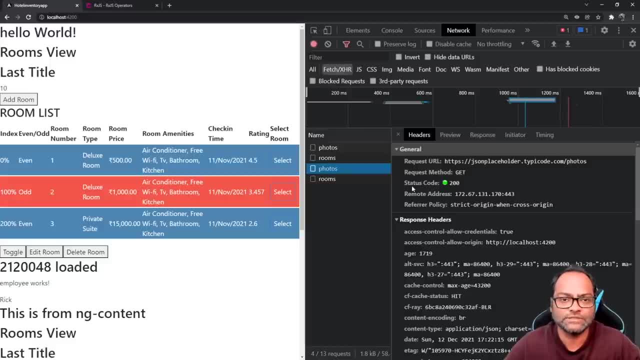 and again, right, Whenever you visit, your user visits the page And in case you are making the same call at multiple places, which is possible. it's not something which you should avoid. It is something which you should avoid, but it's possible that it may happen that you. 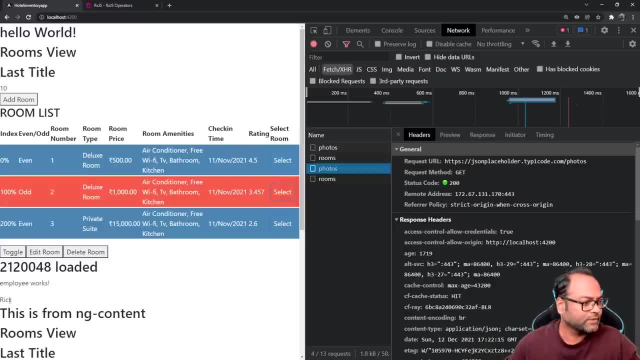 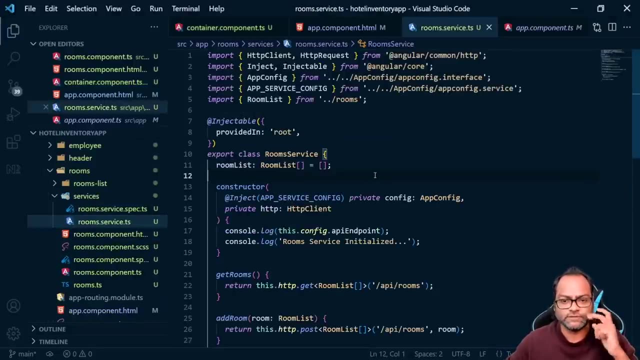 are calling the same API again and again to get some data. So let's see how we can use our RxJS share replay operator to cache this request and make our application a little bit faster. So I'm going to make some changes into room service. 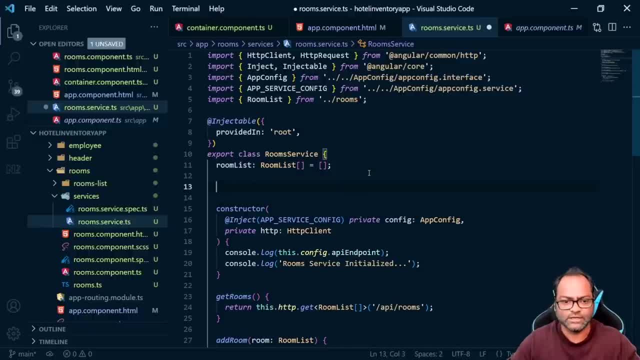 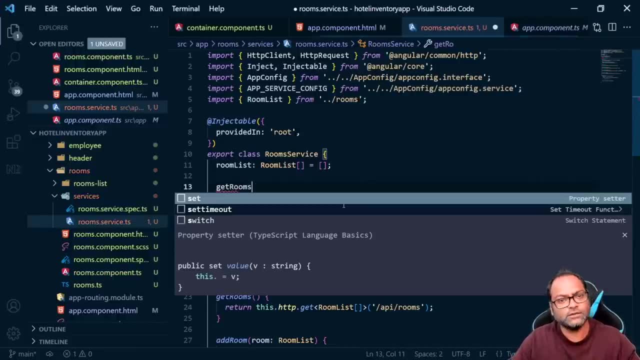 I'm going to use a different approach. Generally, I prefer this. in case I don't have any. I don't need a function, So I'm going to use get rooms, but I'm going to use a dollar, and I'll talk about what this 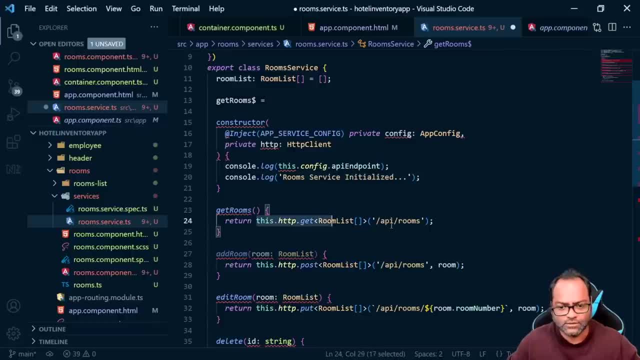 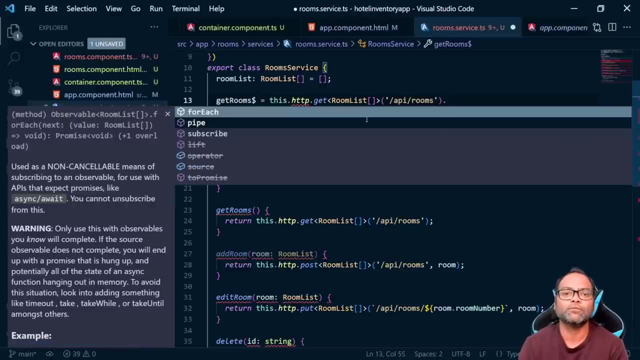 rooms dollar does Okay, And then I'll call this get rooms API. and remember, as I said, we can not go ahead and modify the stream after we subscribe to it. A stream can be modified inside a function. that function is known as pipe. 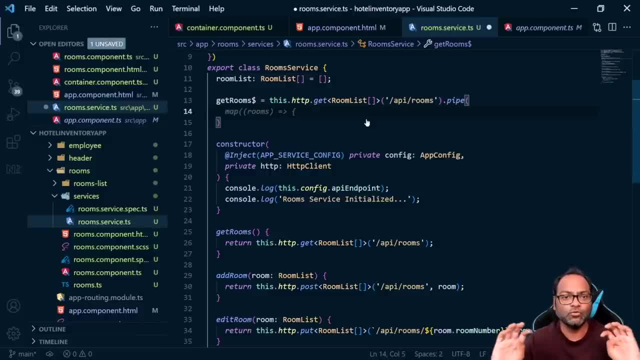 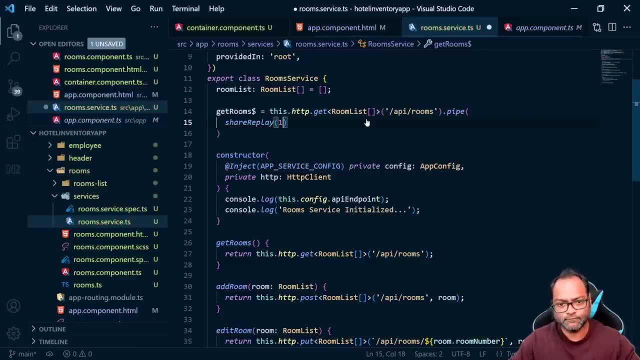 So this pipe is where you can do anything with your data, And right now we are going to call a share replay operator with share replay one, So we are going to repeat or replay the last one record which we have received, And this is done. 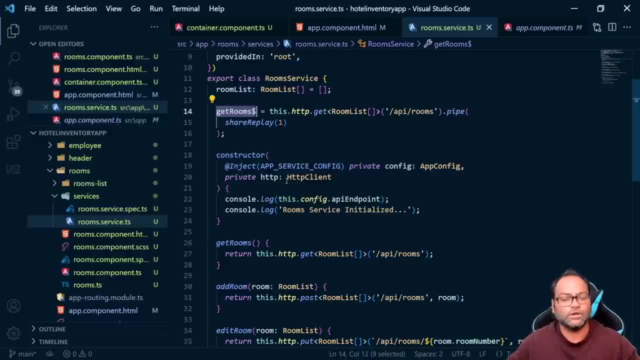 This is the method. Now let me talk about this: get rooms dollar. what we are doing, This is a property, So we are saying this is a property and this dollar is to denote that this is a stream. So, generally, whenever you work with streams, try to use this approach. try to uh use 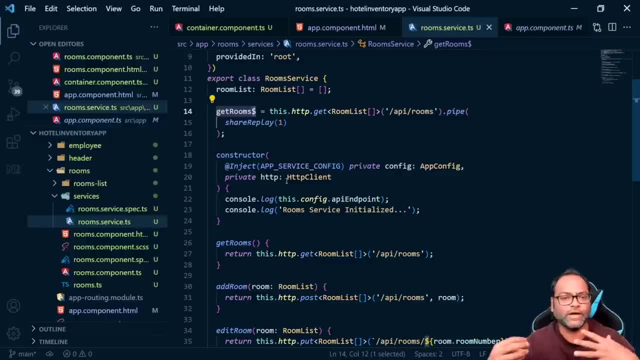 this index, And so you don't need to engineer it, or you don't have to call anything. inside engineering, We'll see an example where we can actually avoid Right Subscription as well. So once you get comfortable with this, it will be easy to understand that code as well. 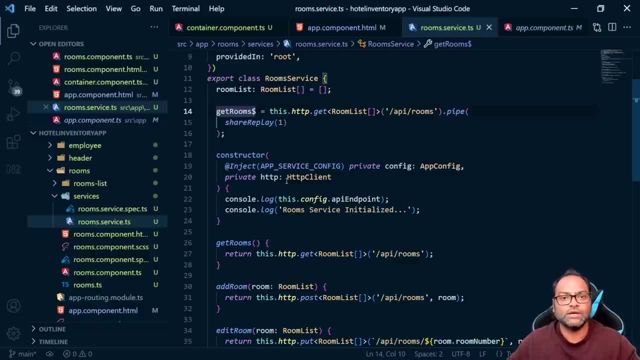 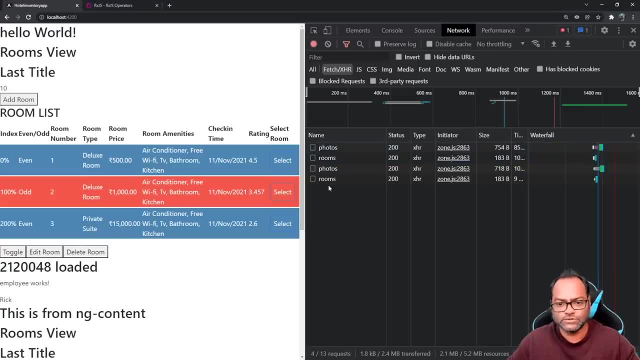 So here we have a property, get rooms, and then we are saying: okay, this is a stream which we get here And so far nothing has changed. We still getting to record, uh, to request, right, So rooms. Now let's go to rooms component or DS here 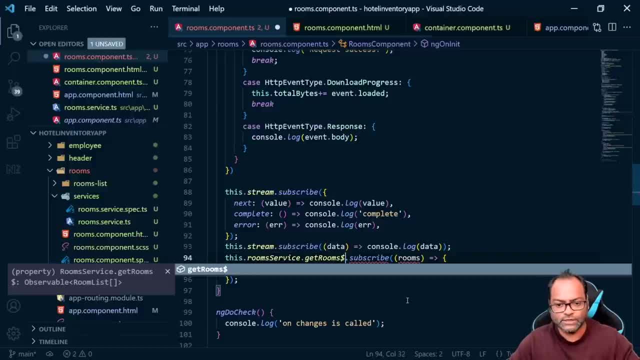 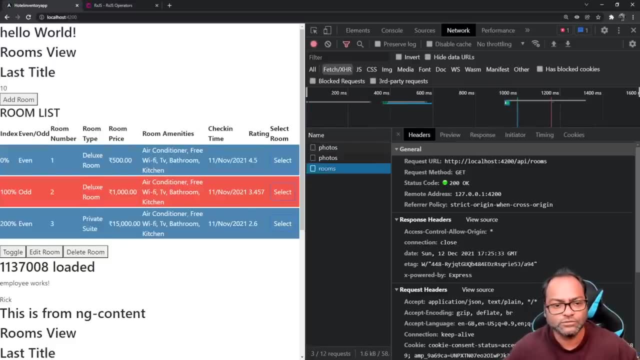 And rather than getting to get rooms, uh, we are going to access get rooms property and let's go ahead and see. Then we are now getting rooms requests only once, but of course we have the data available multiple times because we are caching the first request. 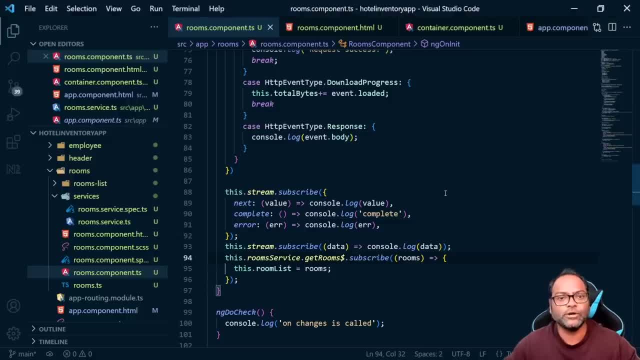 So we don't have to go ahead and make another call. This is something which is really important to understand, because, of course, you may have an application where multiple calls are being made unnecessarily. uh with uh, even though the data never changes. you share play and then you are done. 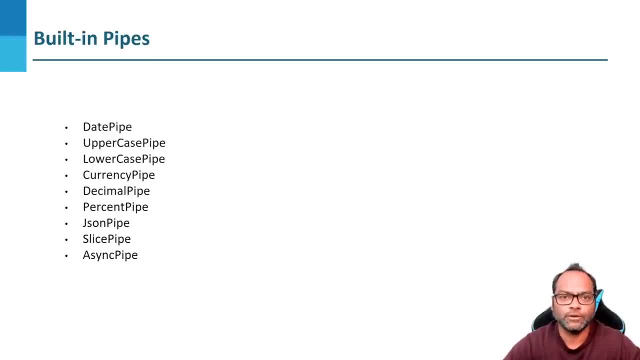 This video, we are going to discuss about one pipe which we had left while talking about building pipes. Remember, we said we are going to use a sync pipe while working with STDP And that's what we are going to explore here. That's why we are back on this particular topic. we are going to see how we can utilize 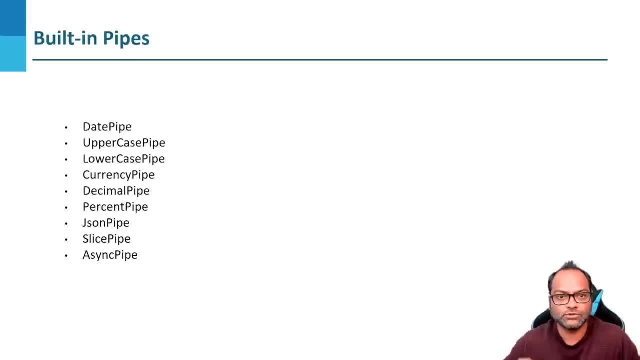 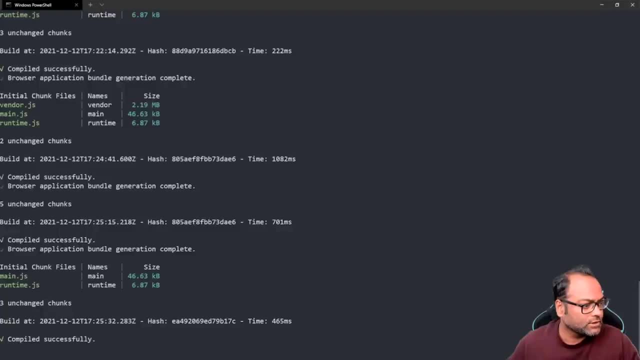 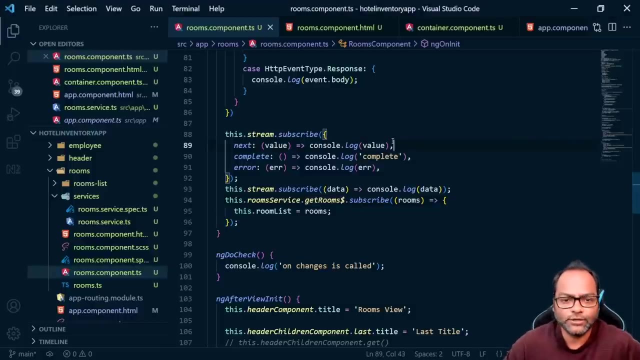 a sync pipe and what's the purpose of using a sync pipe. So this is going to be a little bit uh longer theories plus uh examples, So let's go back to our port. So here, right On the code which we have written, you can see everywhere we are doing: dot subscribe. 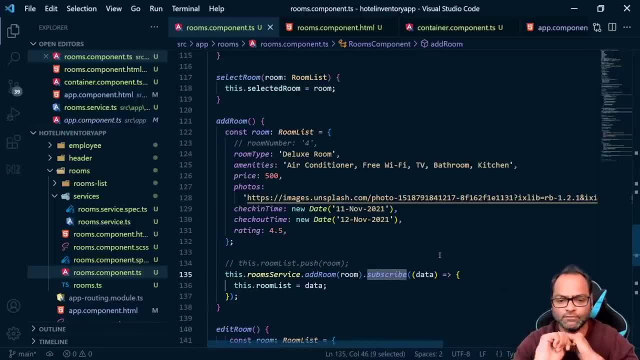 dot subscribe. right, So we are subscribing uh, our uh stream, everywhere. Now there is a downside to this. There is a downside: Yes, To subscribe the streams. let's try to relate this streams, uh streams- to your streaming. services When you subscribe to, let's say, Netflix or Amazon prime. Once you subscribe- let's say, you subscribe to Netflix and you wanted to actually cancel that subscription next month and you forget you actually forgot to cancel your subscription- What happens? You pay the price. 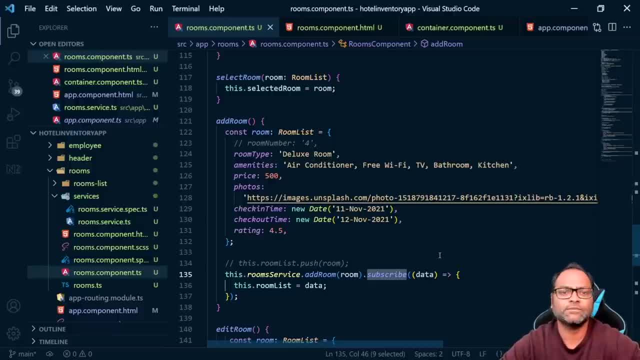 Same thing is applicable here, but here what is the price we are paying? The price is actually performance. So whenever you subscribe to a stream, the streams are active. The standard way is: whenever you subscribe to stream, You should unsubscribe to it. 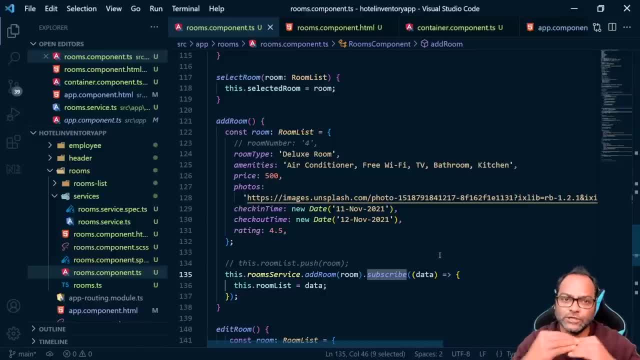 How we can unsubscribe to it. Remember, we discussed about NGO and destroy and we said: NGO and destroy is an event where we can go ahead and uh re, uh, I mean release the resources We can actually unsub. uh, you, we can release anything which we have uh in memory. 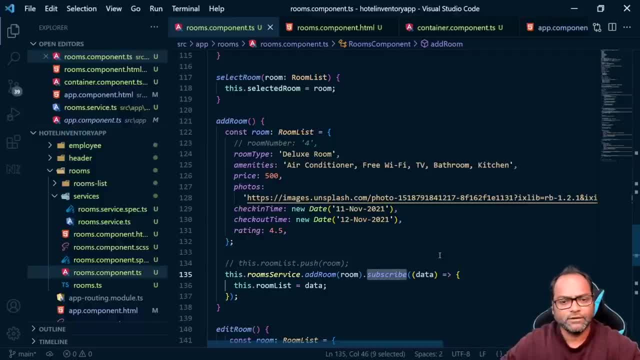 So this is where we can unsubscribe to it, but most of the places we don't need to subscribe manually. It's not impossible, I mean it's not even Uh, it's totally impossible to remove all the subscribe methods. It's not. but yes, there are places, there are things uh uh, there are like operators. 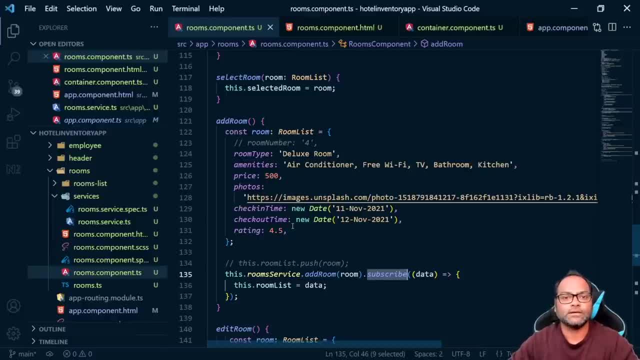 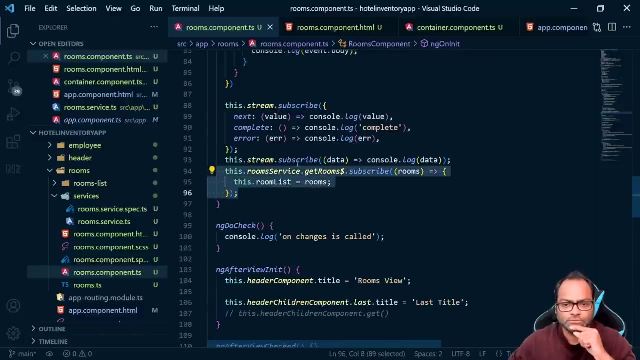 by using which you can. you can do that And, especially in case you want to just read the data, you can go ahead and avoid the streams. Uh, sorry, You can go ahead and avoid the subscription, manual subscription, For example. of course, this one, or uh, we had the photos, one as well. 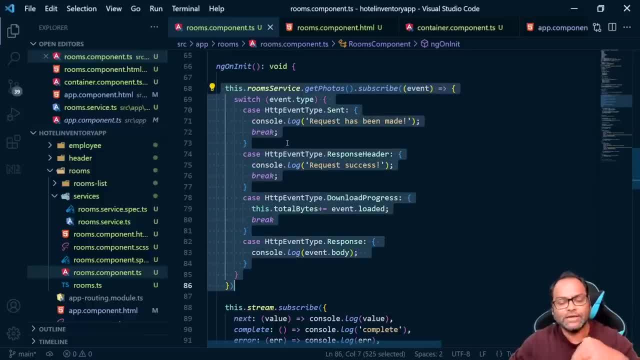 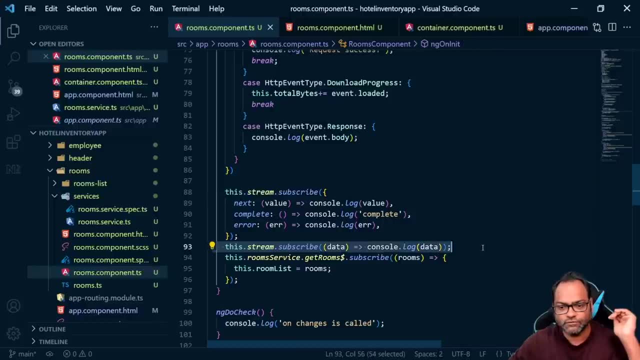 So I mean, of course we are doing here, we are trying diving deep, that, okay, we want to handle this event, this event, this event, but yeah, uh, even in this case, right, So we can just avoid the subscription because we just want you to access the data. 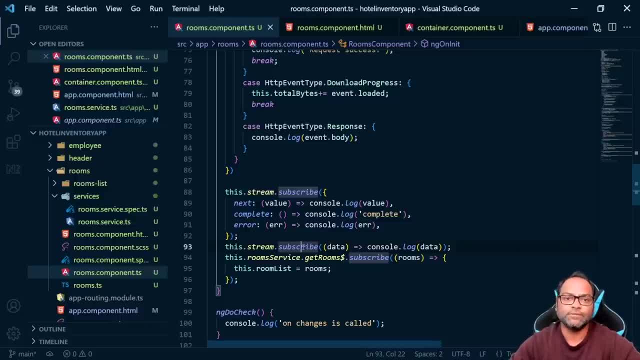 So a sync pipe makes a spot, makes it possible to manage the subscription for us. What, in case, I have to do it myself. So this is how the code will look like, And you will see this code in a lot of places. Yeah, 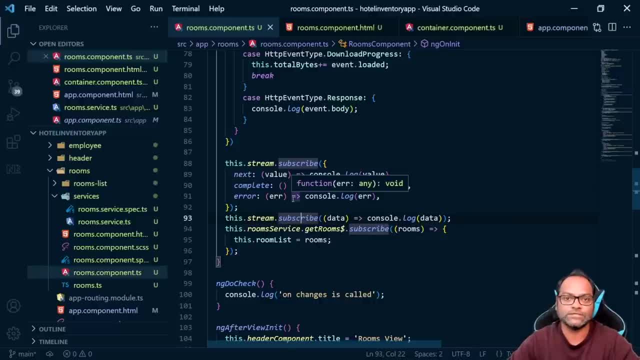 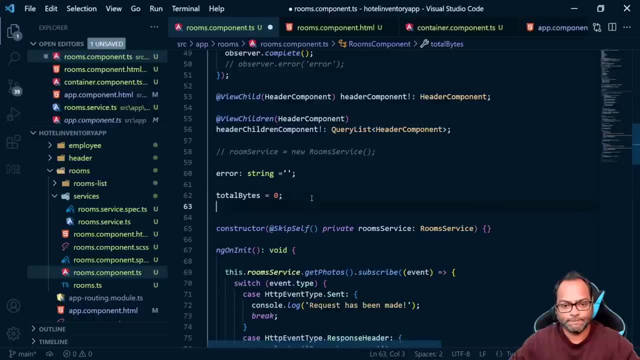 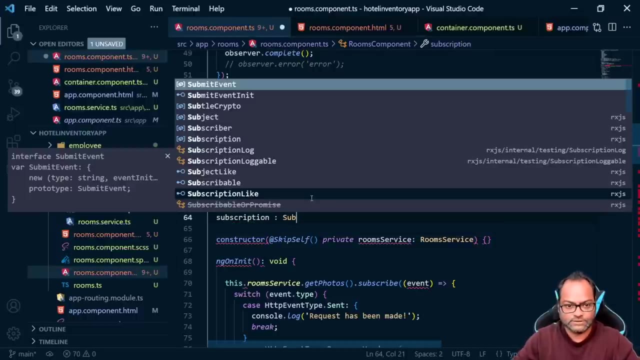 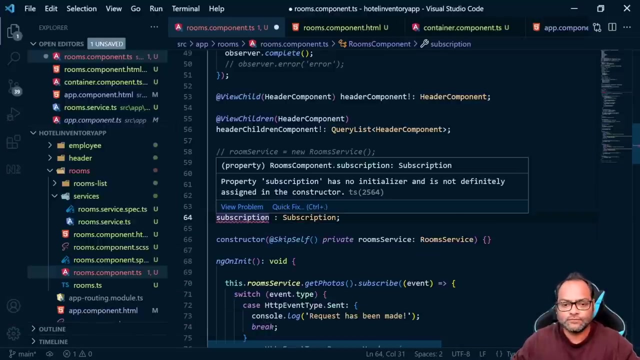 You will see this code in the application or maybe if you get hired to work on any application, probably the chances are high that you will see this code generally be: get an subscription object which is type of subscription which comes from RHS. So you can see: okay, I'll just do this one right. 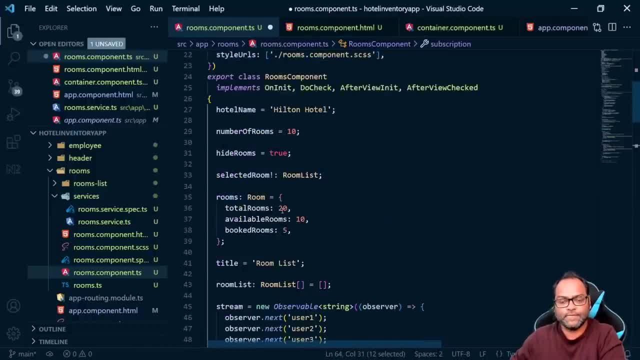 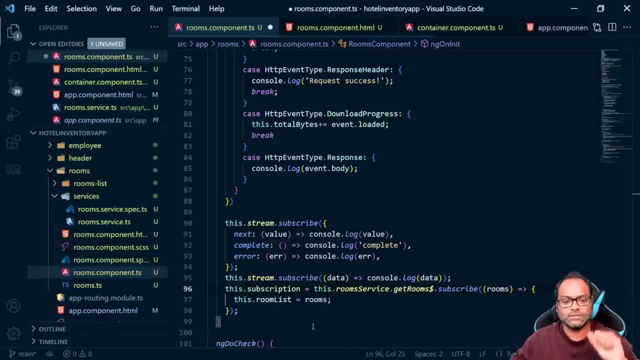 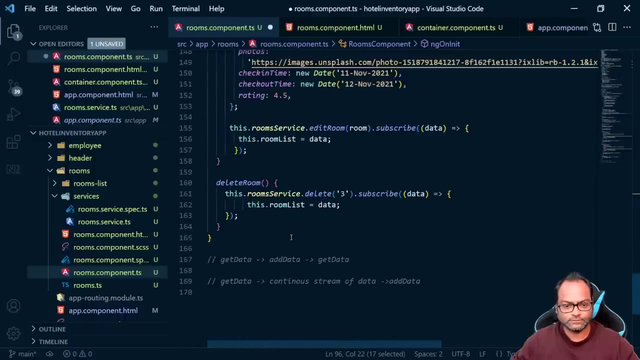 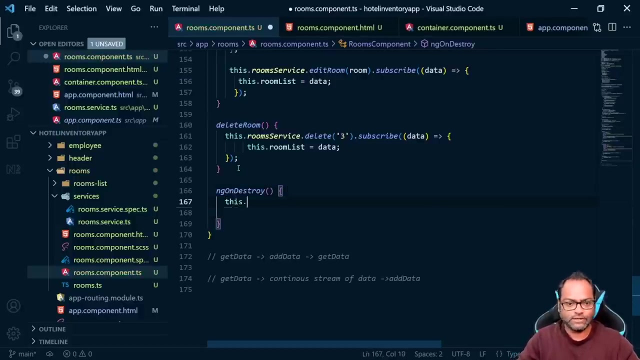 So subscription which has come, which comes from RHS, You can see this and we will ask this. we will use this variable to hold the subscription for us And then I will use ng on destroy and you will find that some code which looks like: 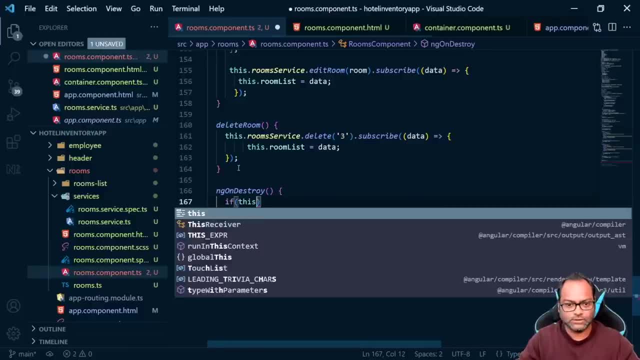 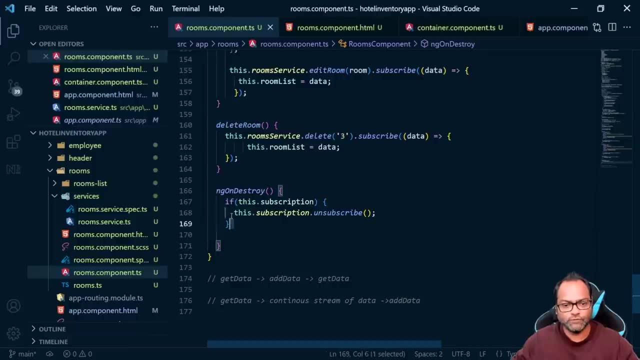 this. So if this dot subscription- Yeah, Yeah, Yeah, It means there are some- there are any active subscription, go ahead and unsubscribe to it. So this is the code which you can find at many places, And this is the way you can actually unsubscribe to an active subscription as well. 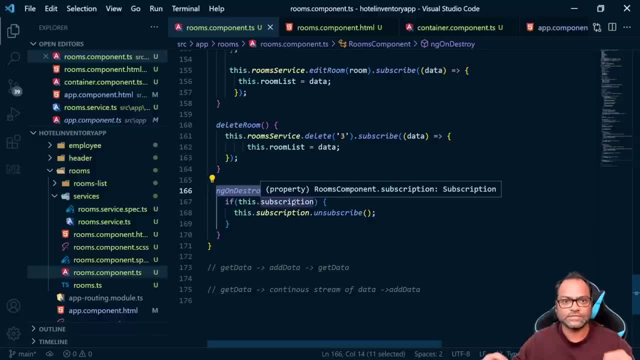 Why ng on destroy, You are saying, whenever this component gets destroyed, just go ahead and destroy the subscription also, because we don't need it, We don't need it to be available in the memory. And in case I want to avoid this, 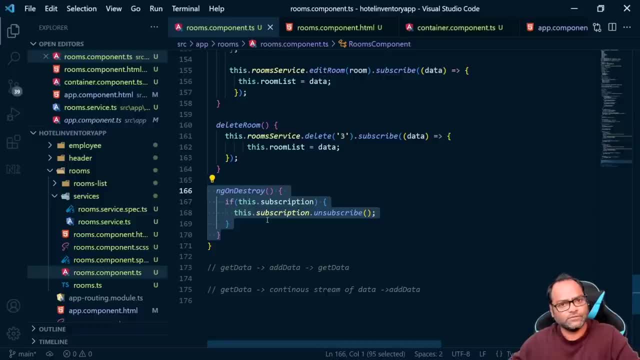 Which I said totally. I mean there is a service. I'll share the code. There is an, actually there is a service which you can use at all the places to actually achieve this, or write this, write your code in a simpler way. 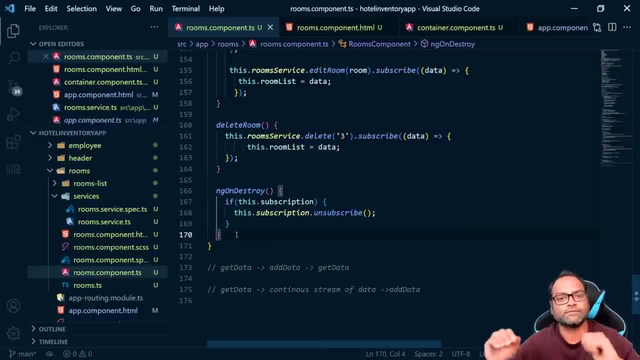 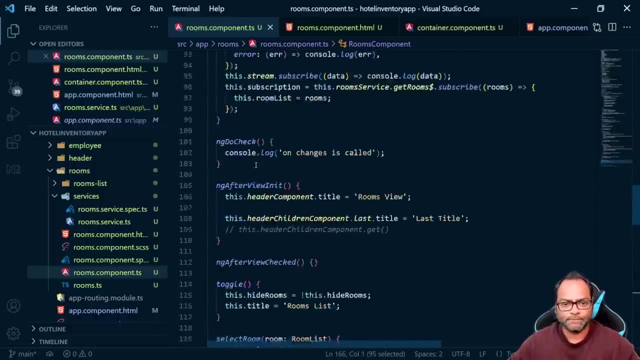 But yeah, I mean I'll share that in future because that that service you can utilize in your real time application here. but right now let's say I don't want to actually subscribe it manually here- how we can do that, so i will remove this and 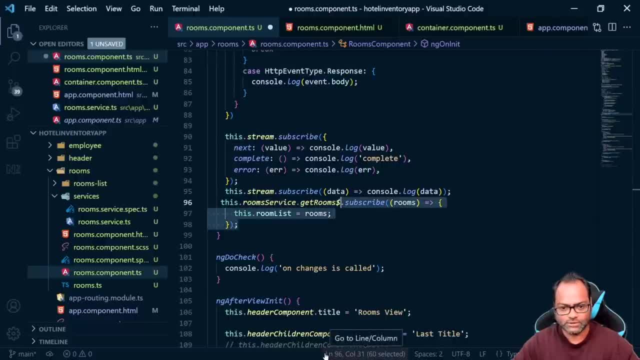 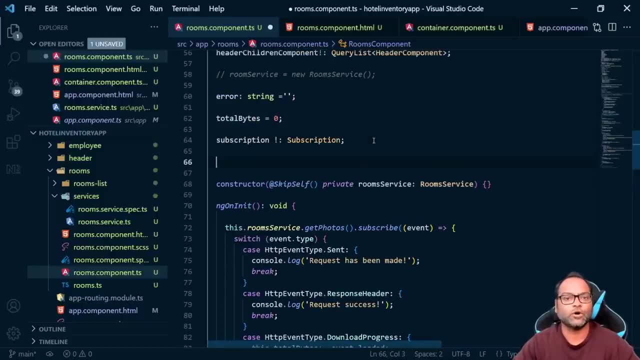 let's use this stream. so i'm going to comment this line because i'll keep it here. but i'll just comment this now: remember the earlier code which we wrote for share replay. i am going to use the same approach here. so i'm going to say: this is uh what. this is rooms. i'm going to say: 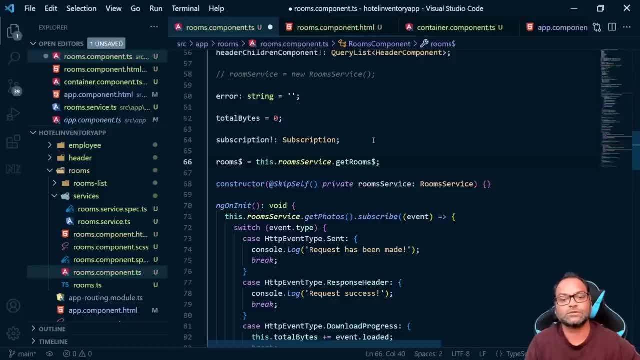 this is the room stream and this is equals to this method. so i'm going to say, okay, this is room stream and actually this data is coming from here. no subscribe method. let's see. once this is done, of course, let's go back to the ui and we will see. okay, there is no data which is available inside my table. 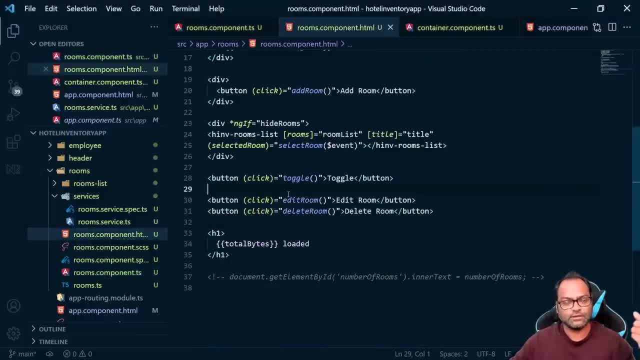 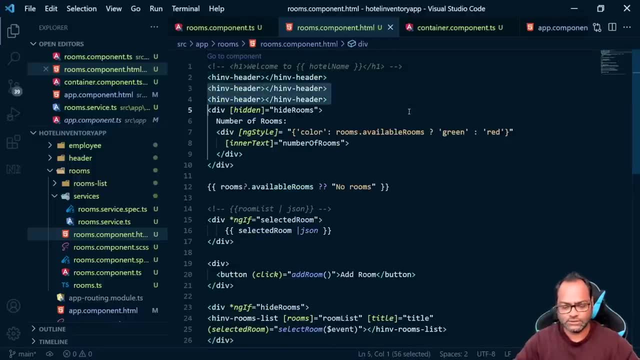 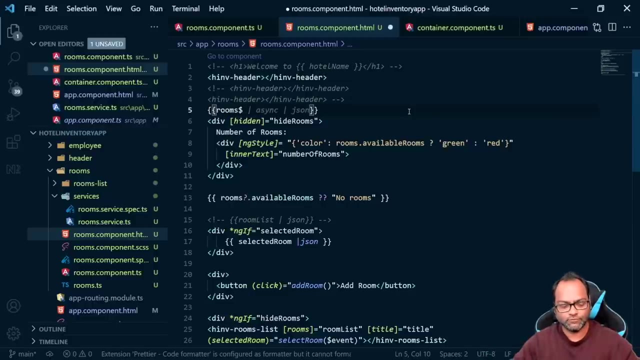 let's go to component and let's try to read what is available here, how we can do that so we can use. i'll just remove some headers here and whenever we have a stream we have to use the async pipe and then i'm using json to display that data. 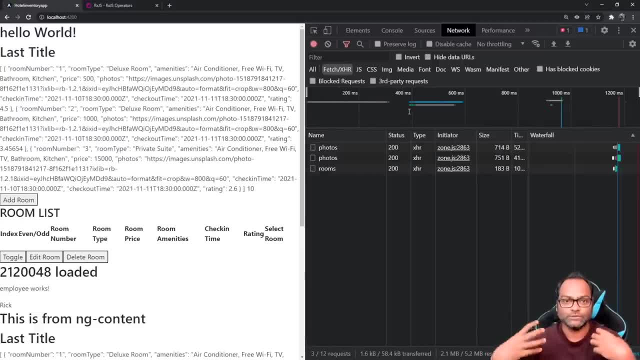 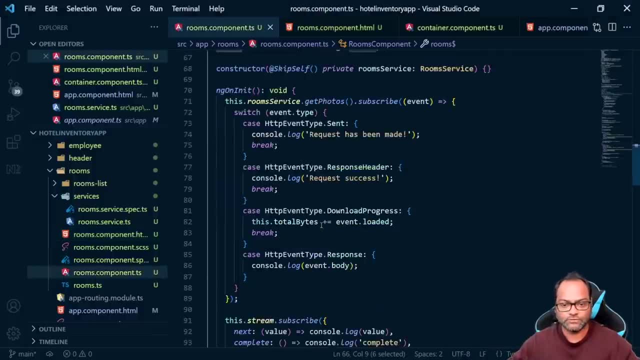 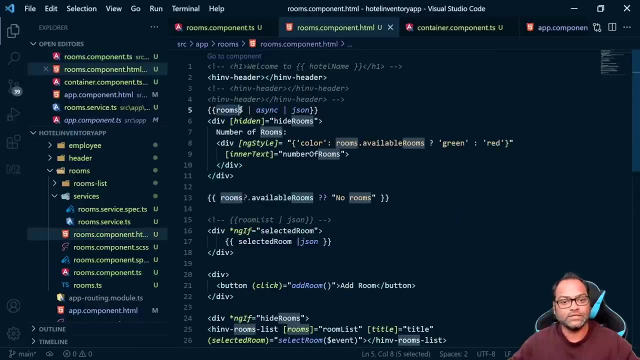 so sync type. what it will do is it will unwrap that object and it will give you the data. so remember earlier, previously, what we used to do is we used to subscribe to get that data out and then read the data. here what is happening is we are passing the entire stream to a sync pipe which will unwrap. 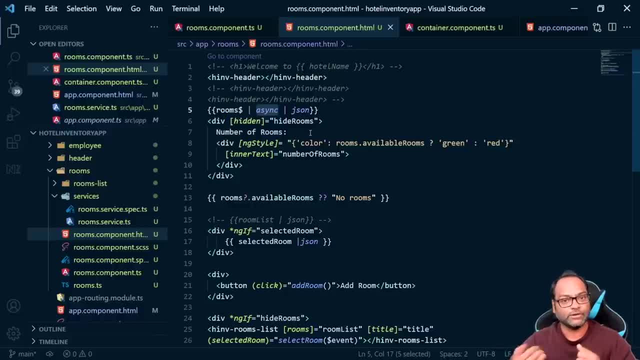 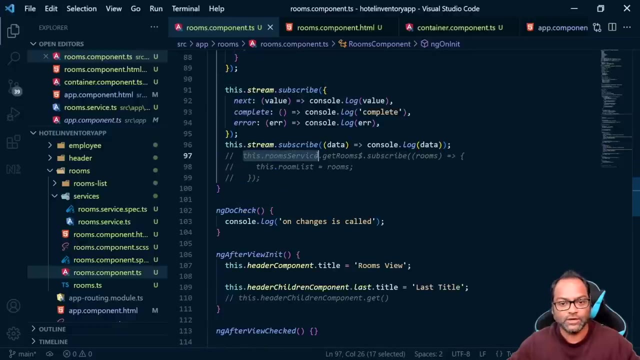 which will unwrap means it will unsubscribe to that particular data and give the data back to us once your ng on destroy is called a sync pipe- will also take care of unsubscribing to that object, so you don't have to write. go ahead and write this code where you say: okay, this is equals. 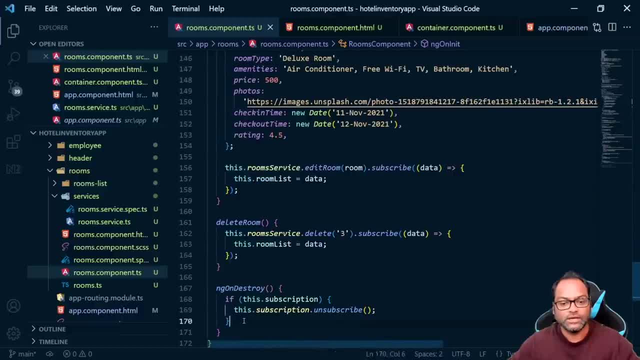 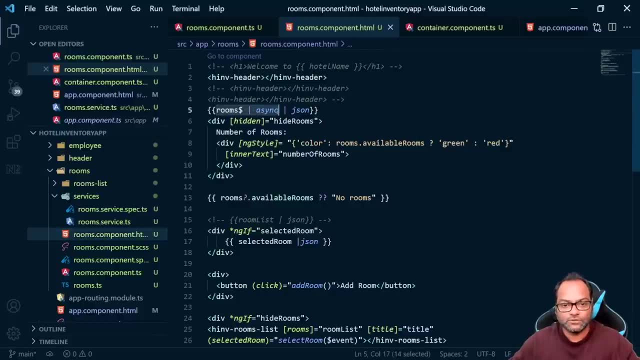 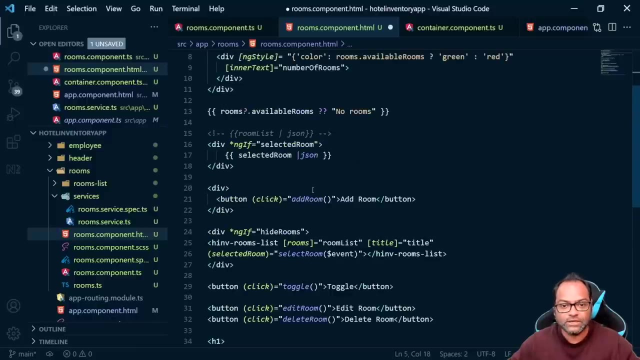 to this- subscription is equals to this, and then unsubscribe in ng on and destroy, so you don't have to write this code by yourself. now let's go ahead and see how we can use it. so i'll just copy this. i'll comment. now we know how my data looks like, and here we are passing this uh rooms data. let's see. 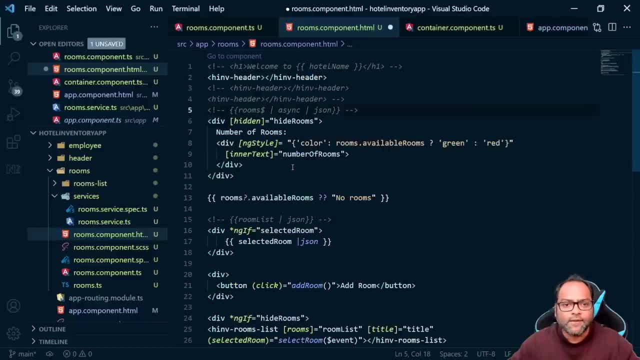 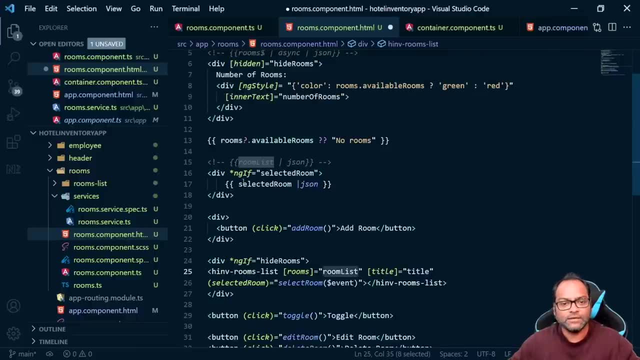 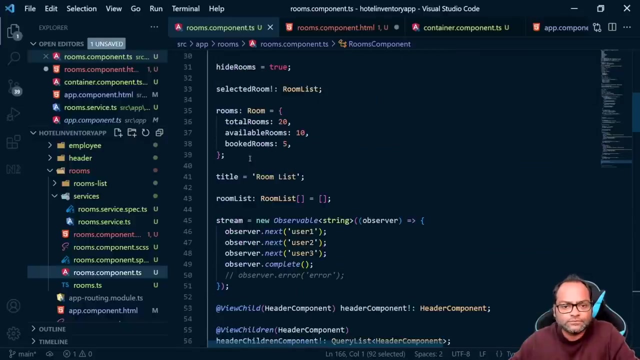 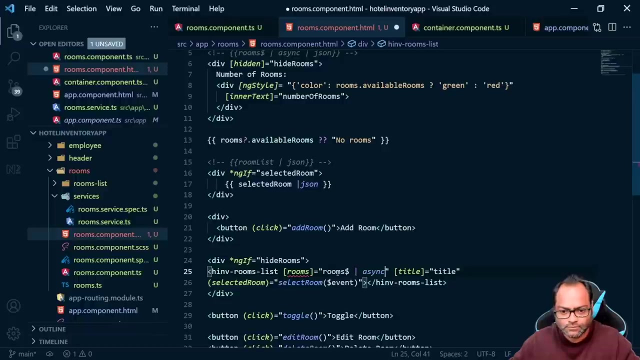 where is my? where is the table here? now i can say, uh, this room stream, okay, pipe a sync. here is it room or rooms, and we will also save ng loves, uh, sing and such, and so in case some rooms in this row and some rooms in this is not going to be so, in case some rooms in the main menu and we are sending rooms to a sync, how do I have to save other in the main menu? 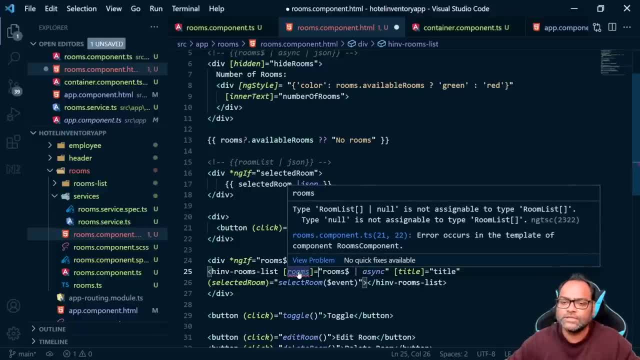 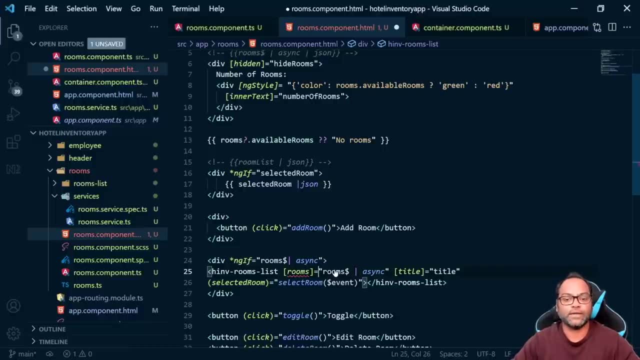 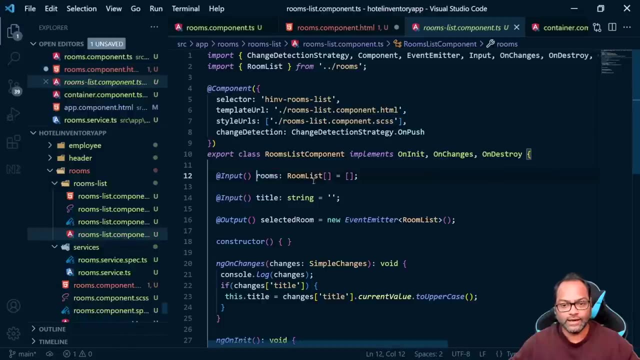 some rooms is available. go ahead and display this and it says a room list of: okay, so rooms can also. uh- sorry, this is a sync pipe- uh can also return null. so that's what it is us telling us right now: that okay, if it is null, i mean i'm not able to assign this to an array, or null, the thing which. 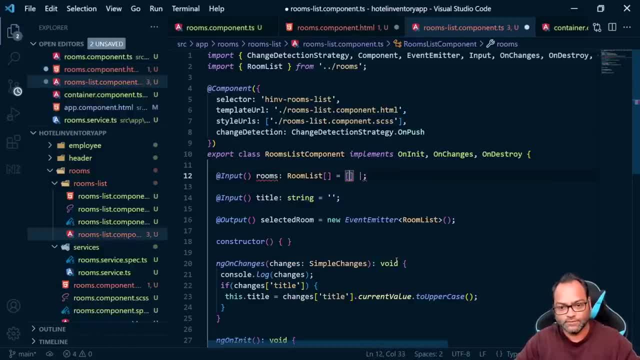 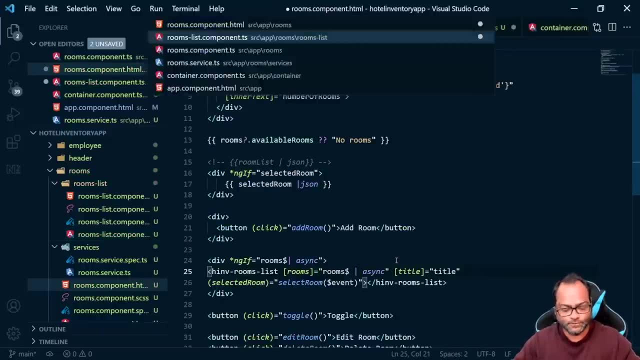 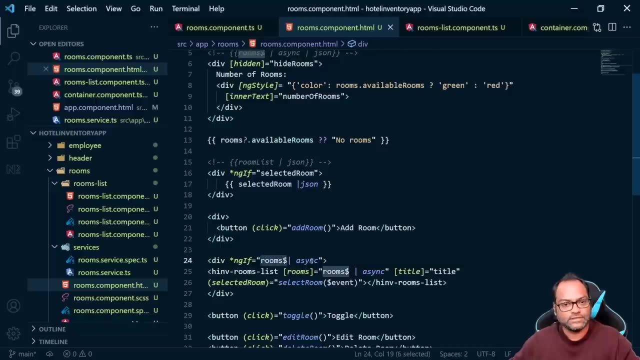 we can do is we can say, okay, this is type of not here, this is type of this or null, and this error will be gone. so now we have- uh, we are checking. if rooms data exists, then only use. but there is a downside to it, so i'll show you. i'll talk about that as well. but right now we have our data, which 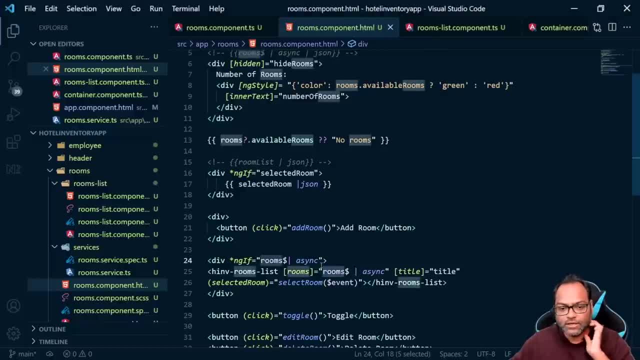 is absolutely fine. right, we are getting the data, but here right now, uh, we are checking this in rooms, a sync, and here also we are doing the same. the downside of doing such or writing this code is we have to- i mean, your sync pipe has to subscribe it multiple times. can we do it at once? yes, that's possible. 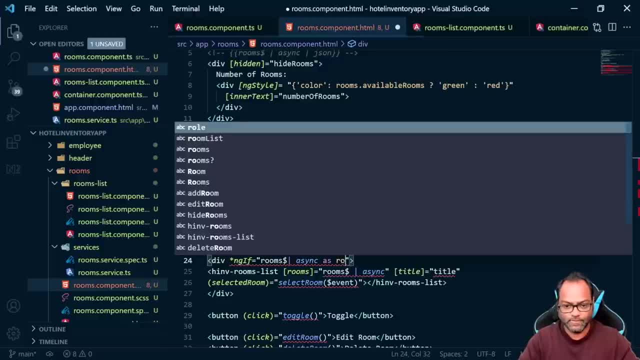 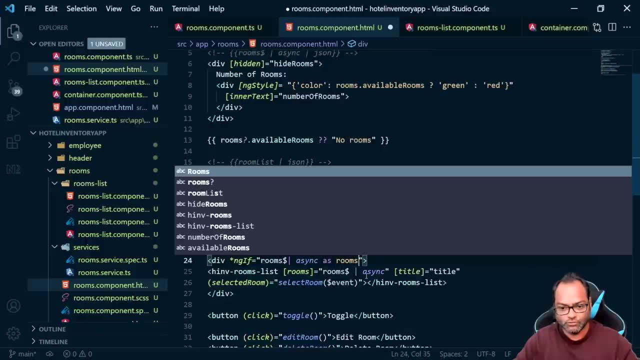 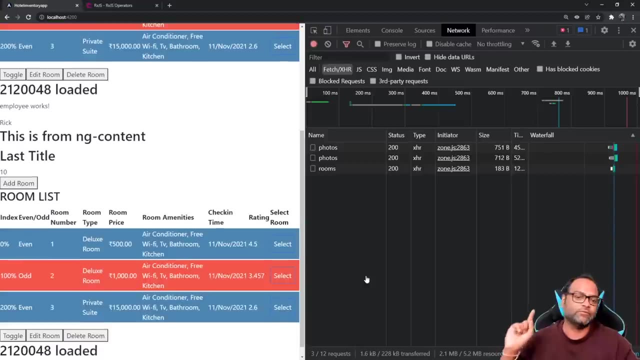 you can do something like this, so you can say: rooms are synced as room and then you can just pass: uh, let's do it. uh, make it rooms and we can pass it here only one, so we have to subscribe only once. let's go ahead and verify our ui and it works no error and everything is as. 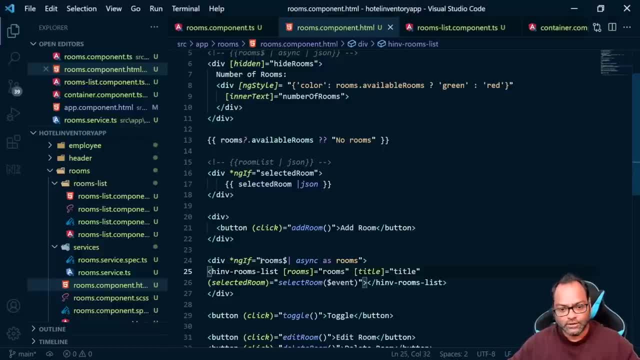 i mean the same as it was earlier. so try to avoid multiple async pipe on the same stream. rather, do this so you can, rather than actually doing multiple passing pipes, you can just say okay as this, and then you can just use that data, unwrapped data down below. so this is how a sync pipe works. 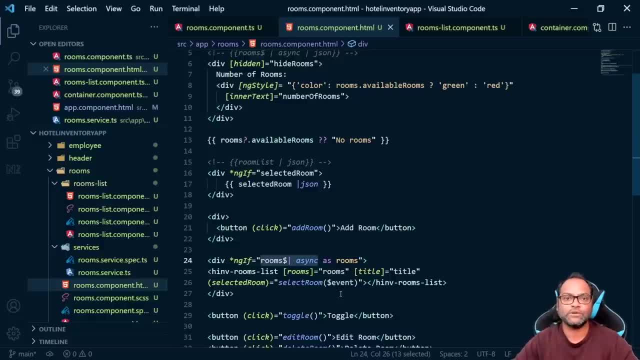 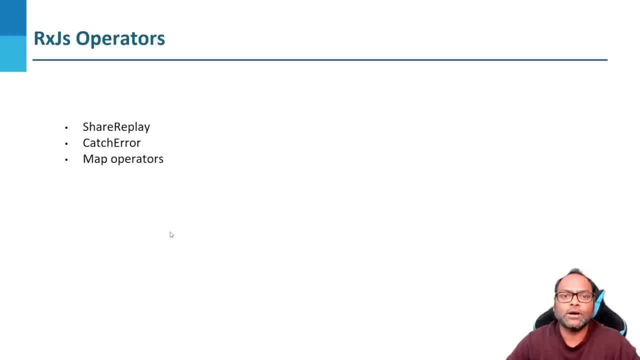 why we discuss about it? because the next operator which we are going to use depends upon sync pipe. let's go ahead and see that. now back to our rxos operators, and right now we are going to talk about the another operator called catcher, and this is why we learned about the sync pipe. so let's see. 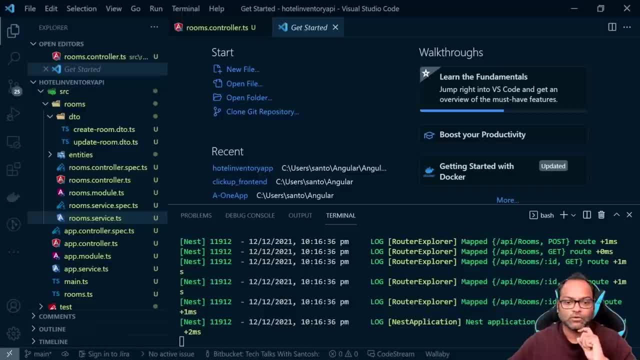 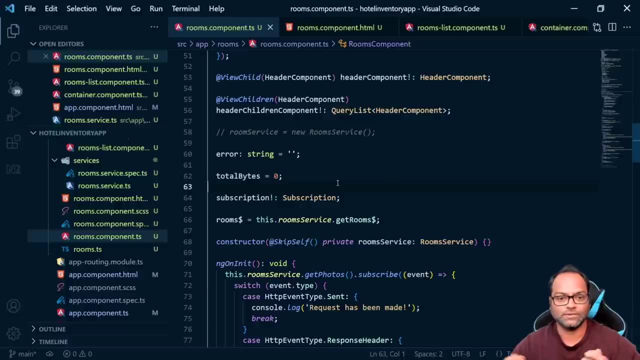 how we can actually handle the errors in our code base. so so far we have written the code, all the fb flow, no exception. that's fine, right, i mean, most of the time you will get the fb flow, but we have to handle the exceptions as well. so here let's try to. 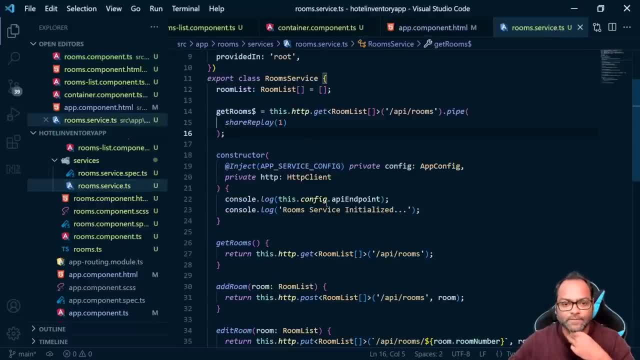 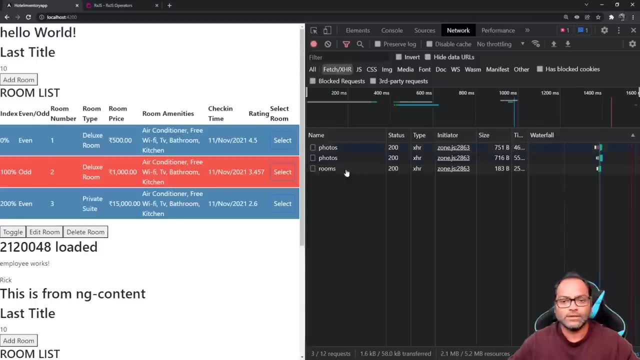 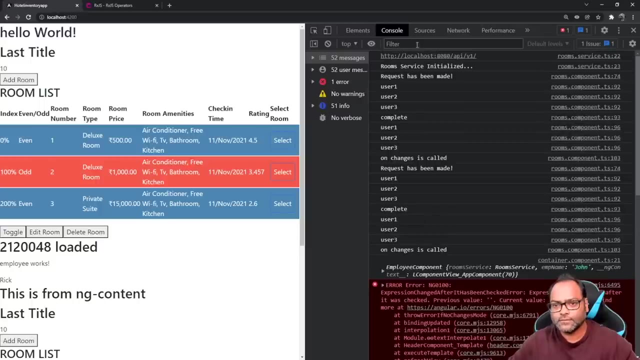 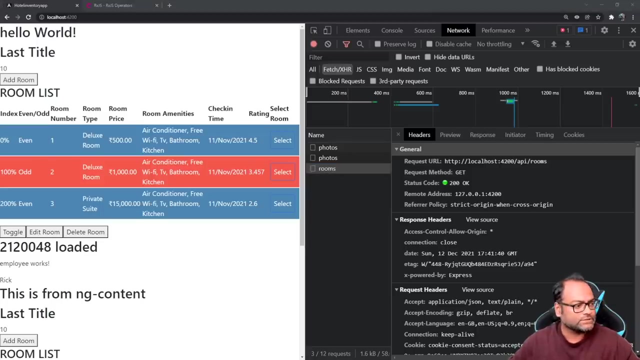 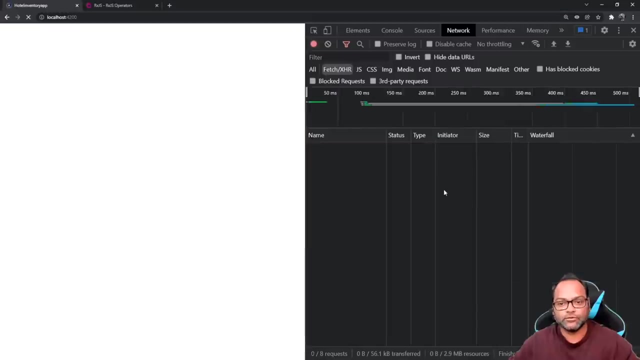 introduce an error. how we can do that. i can just change the api, right, so i can say api slash room and let's see. and we have okay, somehow application still works, but get rooms, okay. sorry, here we are not using the get rooms now, so we will get 404. we generated an error. now how? 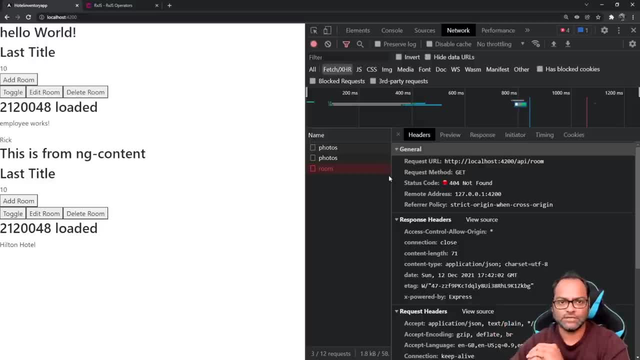 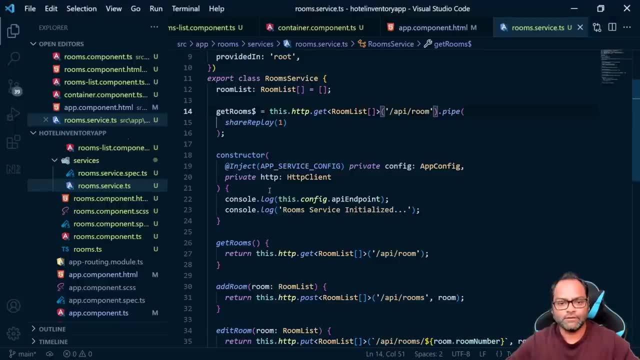 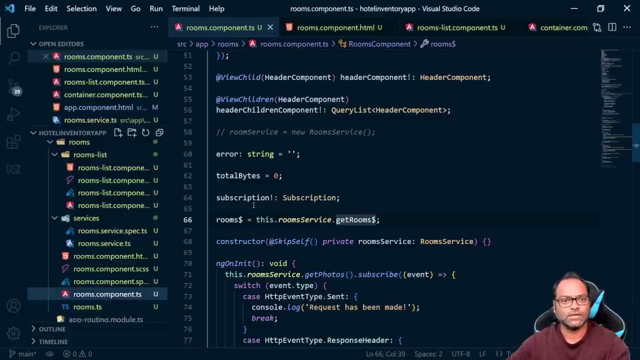 to handle these exceptions. right now we are saying, okay, we have an stream and whenever, like that fish gives you the data, just go ahead and display them. let's see an example where we can also handle the exception, so you can handle the exception inside service as well as in your component- the best. 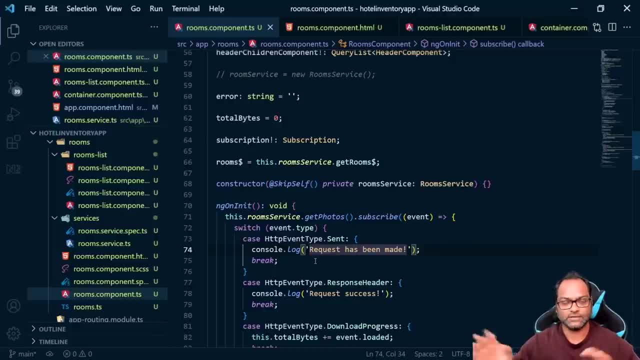 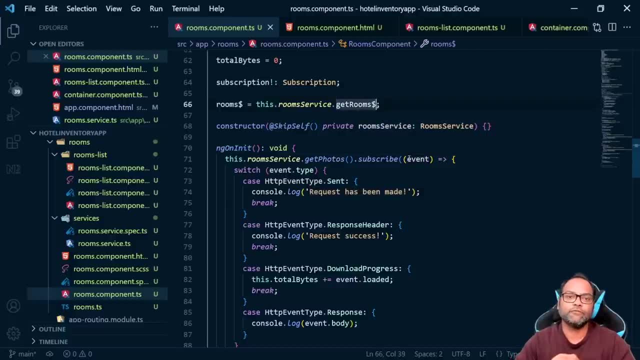 thing would be to use something like back decking in the last five years when they used that to jealous NGRX, which is like advanced optic, which is not part of this. but yeah, let me show you how we can handle exception here. so this stream: as i said, we cannot modify the stream after we subscribe to it. 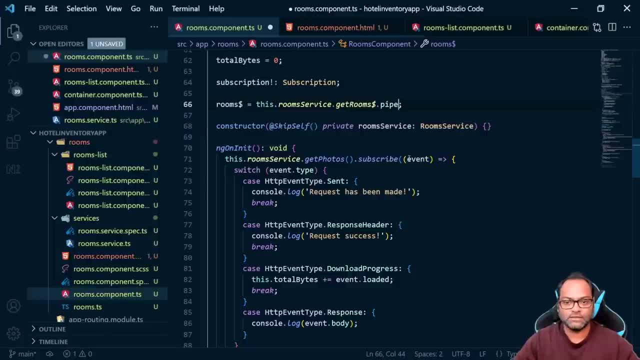 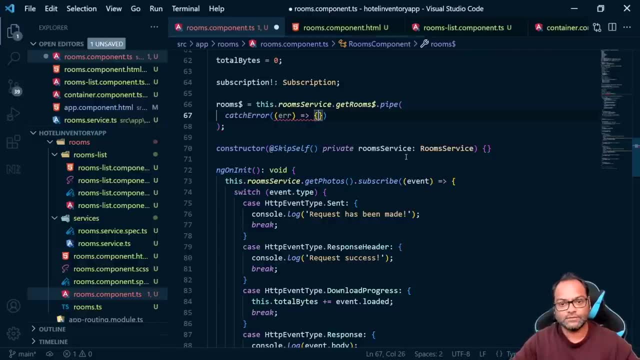 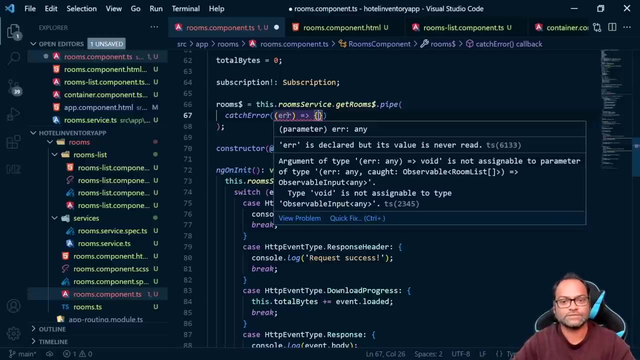 but we can modify it by using pipe. so we will apply the pipe and here i'm going to say, uh, catch, error. this is the NGRX function which we have and we will handle the exception here. but it says, okay, there is some problem. so it says that it declared, but right now we are not using its. 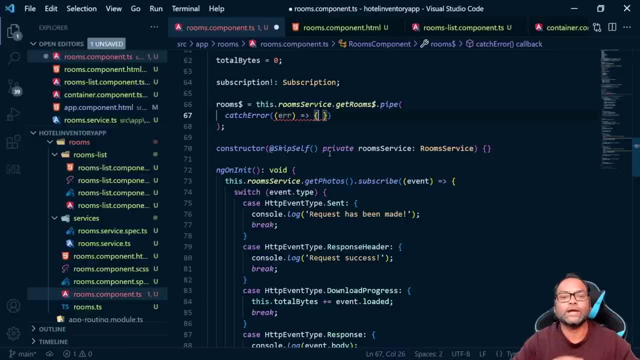 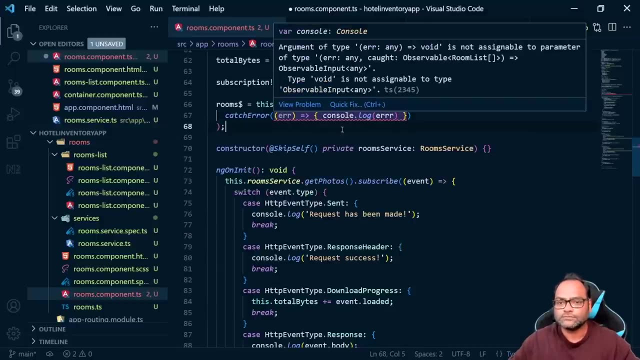 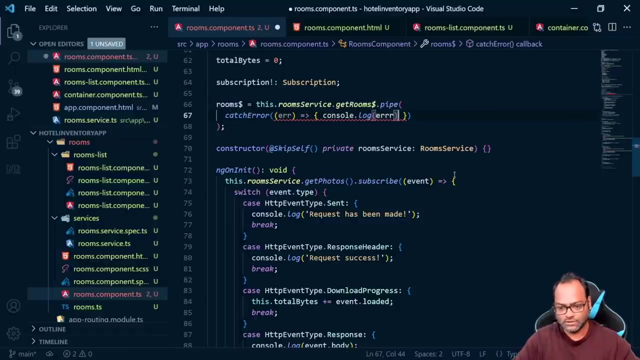 value. let's try to use the value and to do that. what we will do is we will say: right now, let's to consolelog and we'll say error. and it says: array of void: okay, so it accepts room list. uh, parameter, right. so we can say, okay, do this, capture the error and return off. 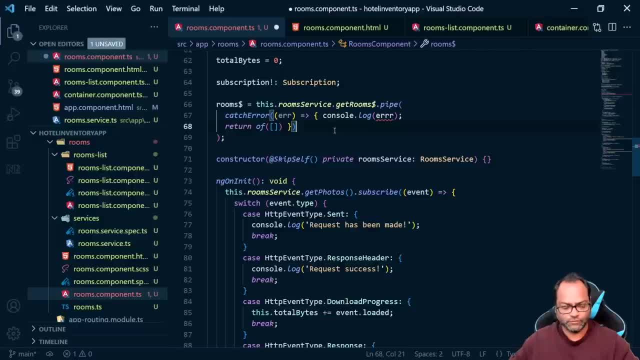 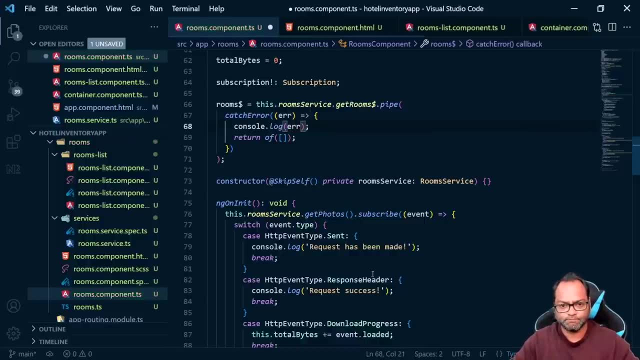 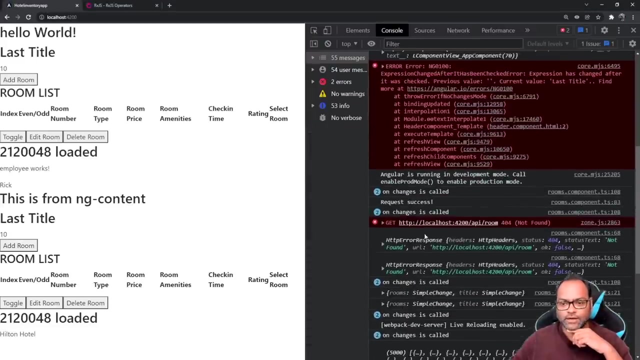 this. i'll explain what we are doing here. let's format and we have an extra error. okay, so we are handling, uh, we are. we are saying, okay, this is uh, log the error and then just return the empty array. so let's go ahead and see: okay, so nothing here. let's see the console and we have the uh error. 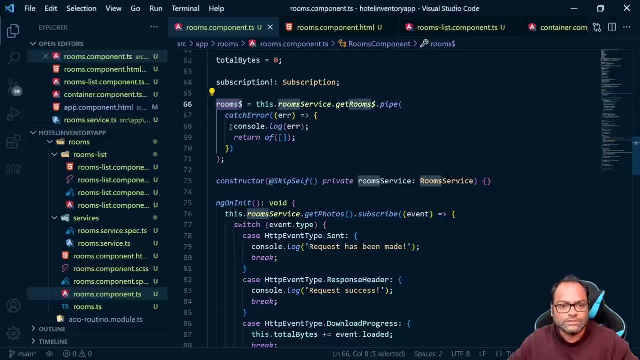 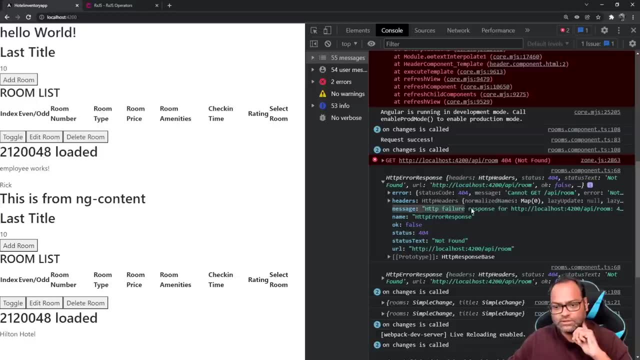 which is http line number. let's see line number 68. yeah, so, line number 68. we have error, http error response and it says: okay, this is the message, right, so this is the actual message which we have. now what we need is we, let's say, we want to display this particular message we want to show. 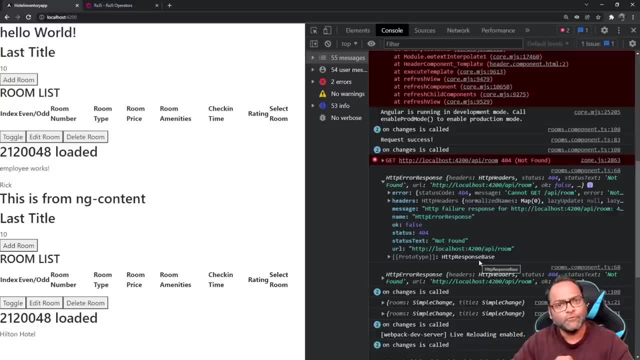 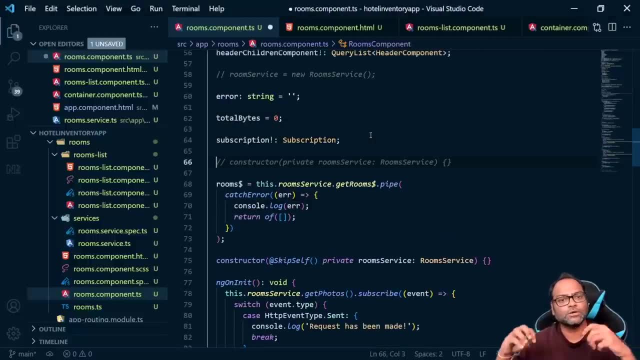 okay, this, this is the actual error which we have received. how we can do that? i'm going to use another uh type which is available in RxJS, which is both observable and observer, so i'm going to create an error string which is available in RxJS, which is both observable and observer, so i'm going to create an error. 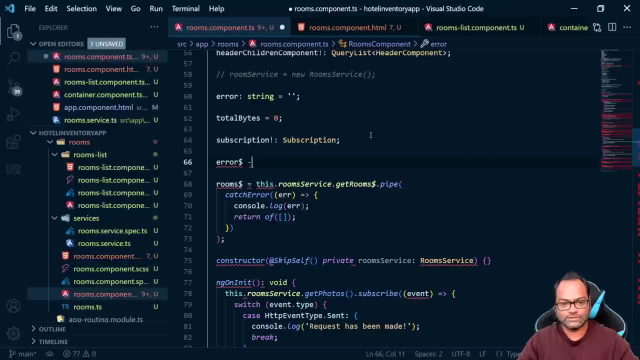 stream and i'm going to say this is a type of subject and it is sorry, it's just type of subject and which is type of string, sorry. and as this is not initialized, i'm going to say okay, this is incation operator, which will avoid that particular error. 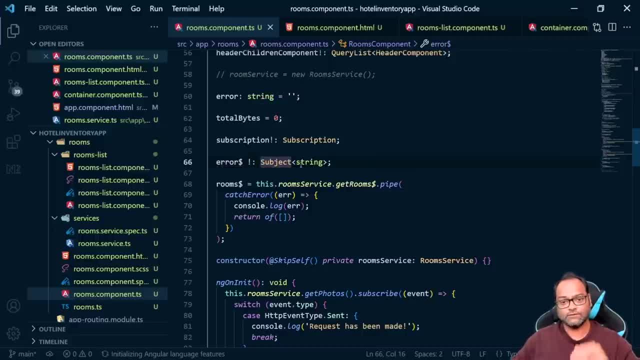 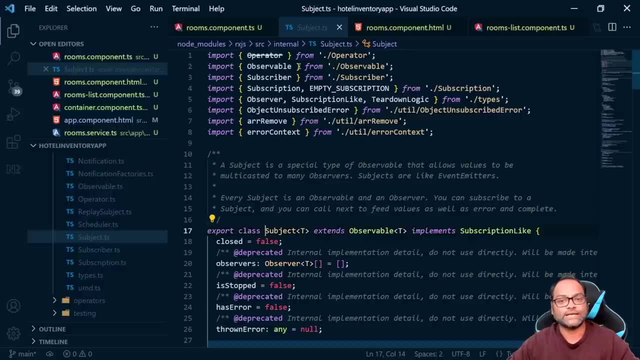 sorry, and as this is not initialized, i'm going to say, okay, this is type of subject. now let's see what is this particular subject is. as you can see, it is coming from RxJS, of course, and this subject is actually base class for all the uh. 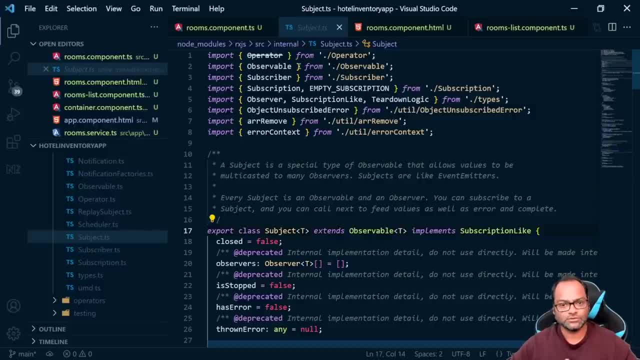 different uh uh streams which you get. so it's a uh like, uh, what you can say. it's a base class, right, for all the type of streams which you get, this is the best base class so you can actually create a subject. and then there are different types. 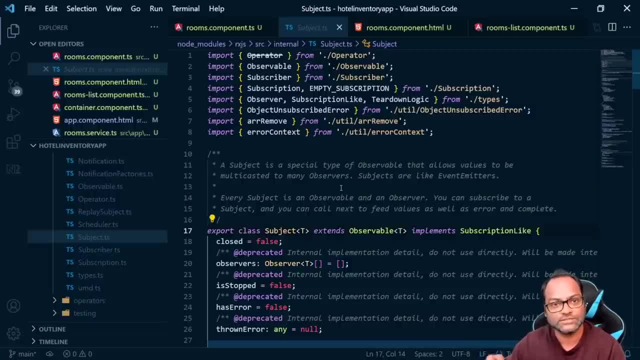 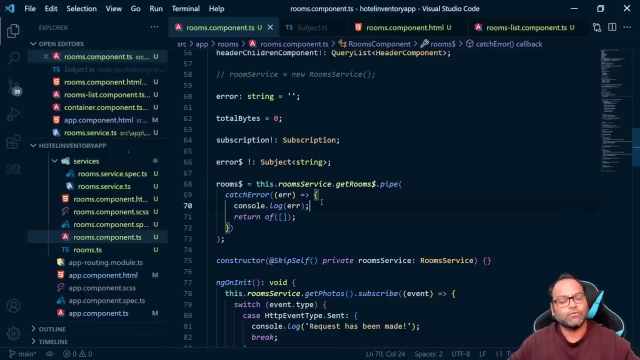 of subjects which also exist internally. angular also uses subject at lot of places. so here, uh, what we have done is we have created, uh, this subject. and now, here, what i'm going to do is i'm going to say, okay, this dot, error dot. i'm going to call a. 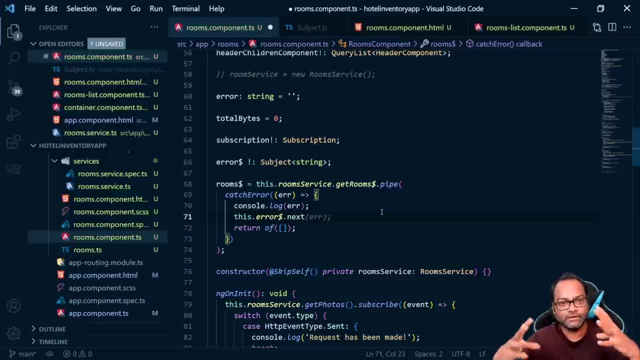 method called next remember. we said: whenever we we saw an example of observer, we said there are three methods which exist: next, complete and error. so we are going to say next, error. and whenever we get the uh, new error value, we are going to subscribe to this. so we are going to say: 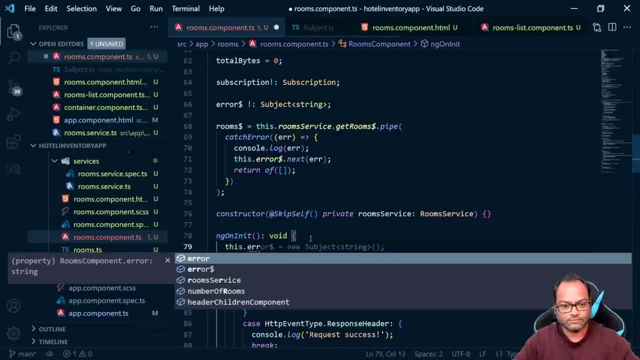 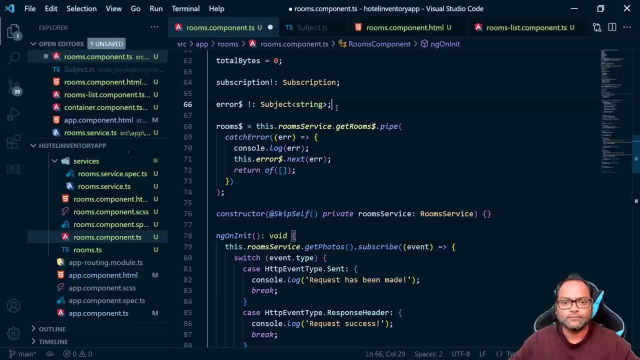 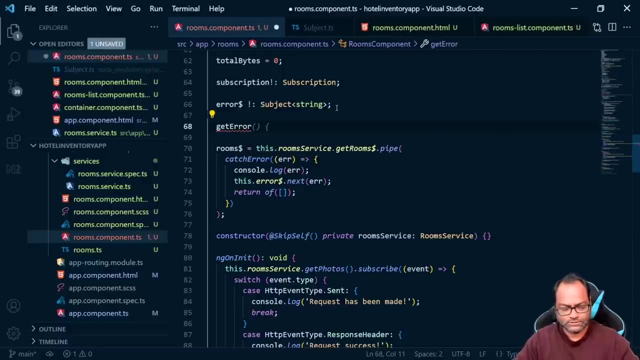 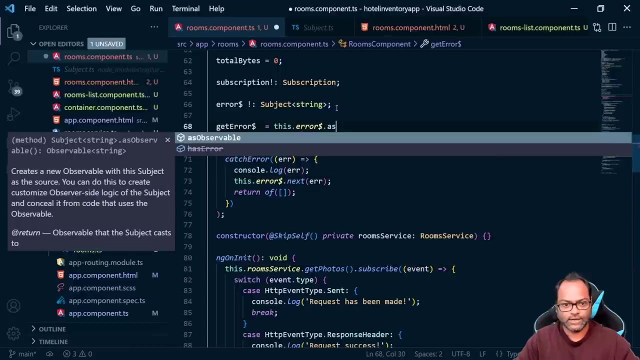 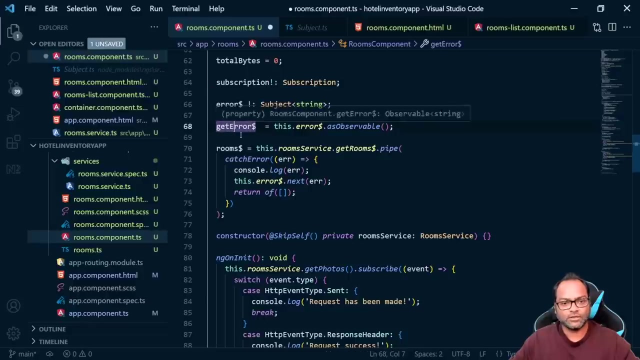 here this dot. we don't have to. let's see, let's do this dot. error stream dot as observable. so this is my subject, this: get error or let's make it. i'll keep it. get error as of now. i am saying i'm going to subscribe to this. so this is this. 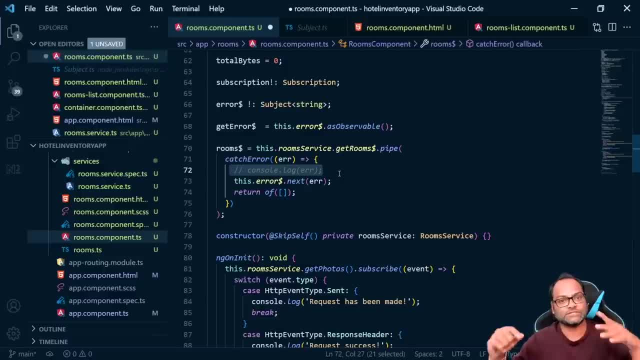 active stream. whenever there is an, there is an error which is erased, i'm going to push this error. you generally should not write this code inside your component because there is a drawback: whenever next gets called, you are your change detection is going to run again. so that's a. 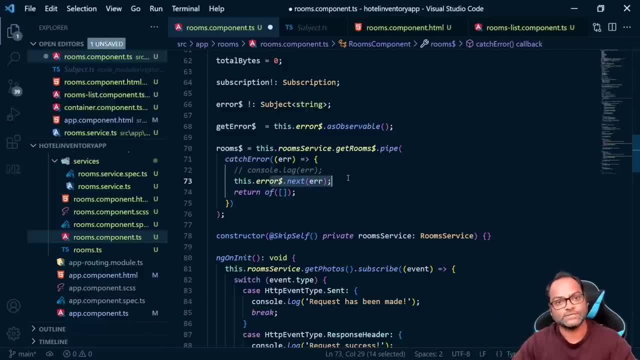 drawback, but of course, you should learn about this- how to do exception handling as well. you can move this to your service. you can move it to another common place, wherever you want to. but yeah, now we have this error which is available, and now let's go ahead and see, so i'm going to save this. 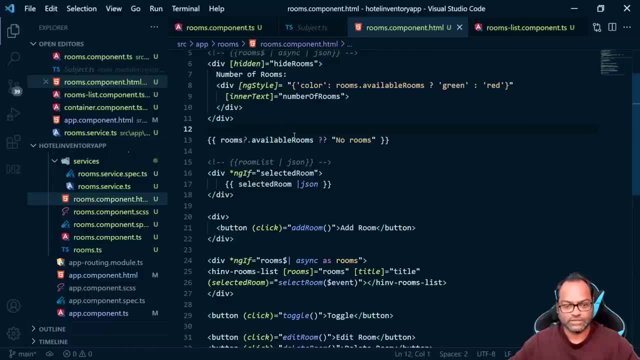 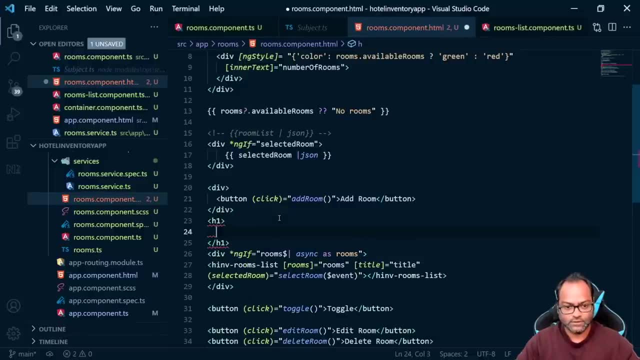 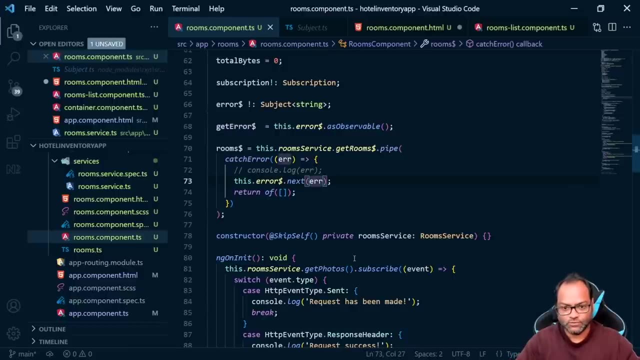 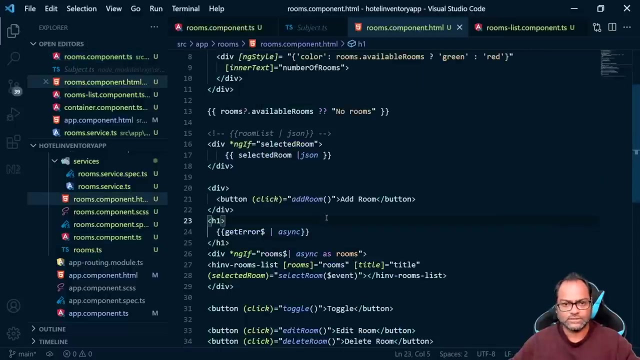 and going to subscribe to this error just above this. and uh, here i'll say h1 and get error pipe sync and what i'm going to do is i'm just going to take message out of it, right, so we don't need to display the entire error. so let's see how the ui looks like. 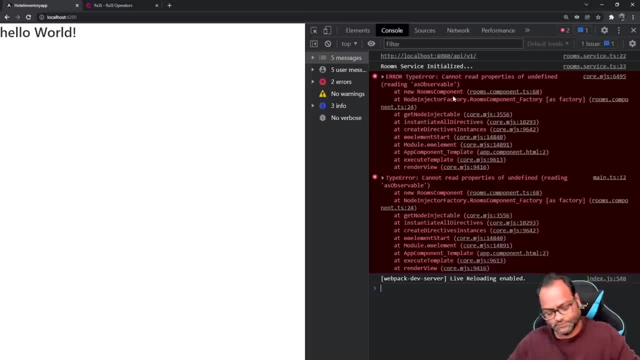 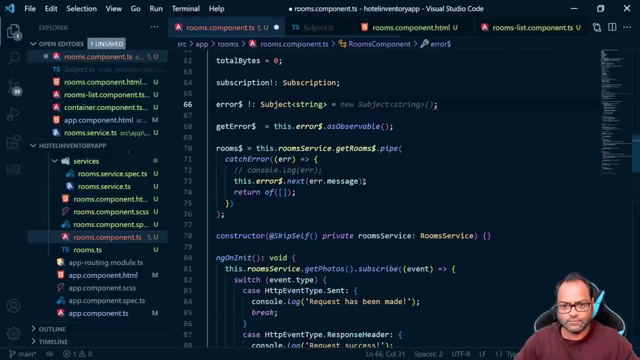 and okay, there is some error: cannot read properties of undefined. okay, probably i'm missing something. let's see. okay, new subject. this is how it should be. actually. we have to create a new subject of type string, and this should fix the issue. now we have, of course, everything is working fine looks. 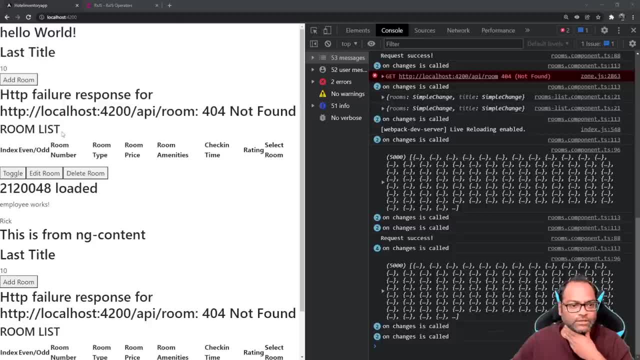 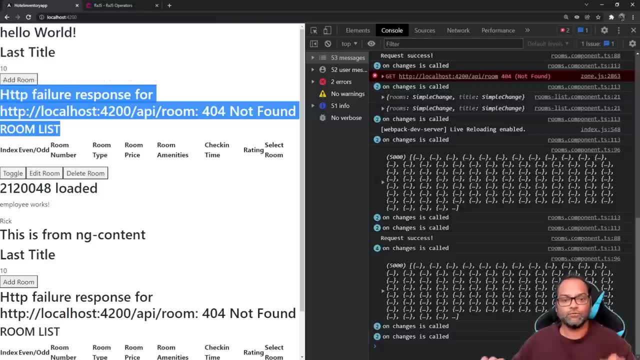 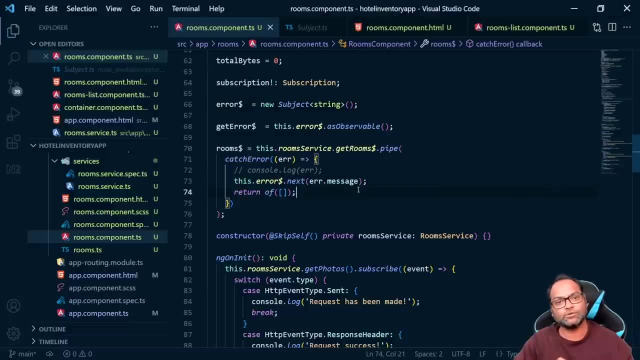 like everything is working fine, but you can see you have error code available here, so it says your error message has to be failure response for this blah, blah, blah, which is everything available now. so what we are doing is, whenever there is an exception, now we are handling that error, we are handling that error and then we are subscribing to that. 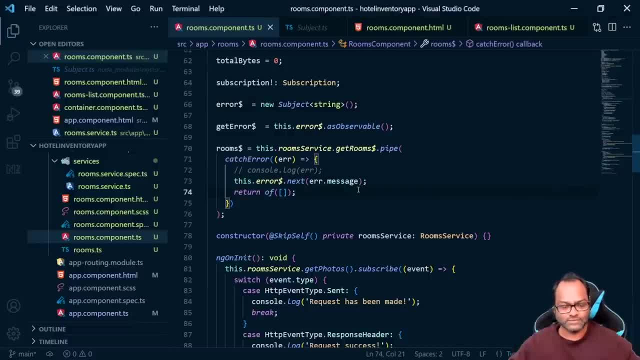 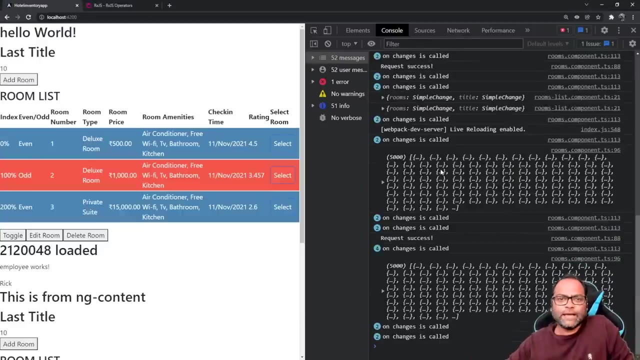 error as well. we are saying: okay, in case we get the data, that's absolutely fine, but in case i get the error, just go ahead and display the error as well. you can customize this error based on your requirement. now let's go ahead and fix the url and our data will be back. now we don't have. 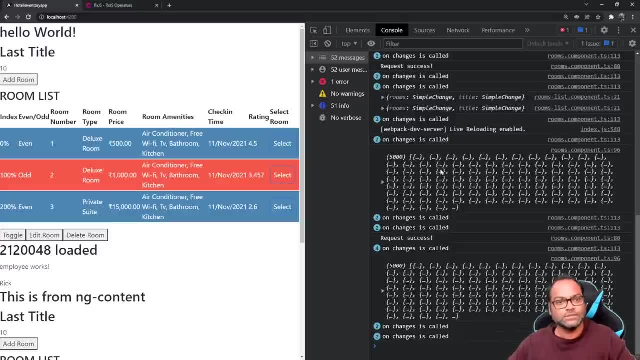 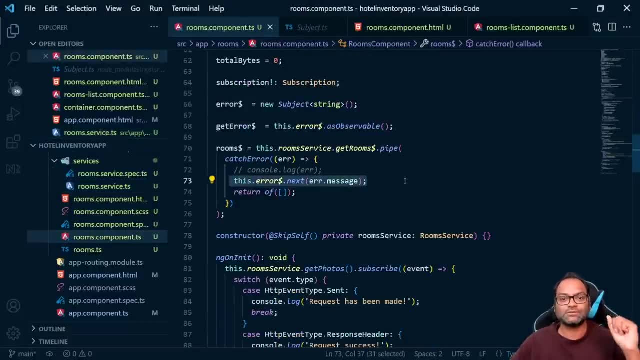 any error. so nothing, uh, no error will be subscribed to right. so this is how you can use catcher and, yes, just make sure that, okay, you are not doing not writing this code in your component. this is just an example. you can do it inside service. we will see an example of where we do the component interaction using service, where we are going to. 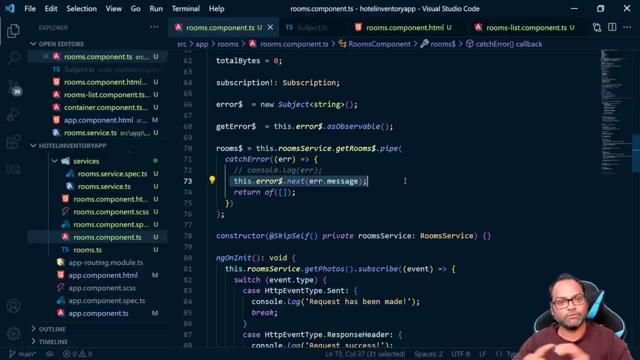 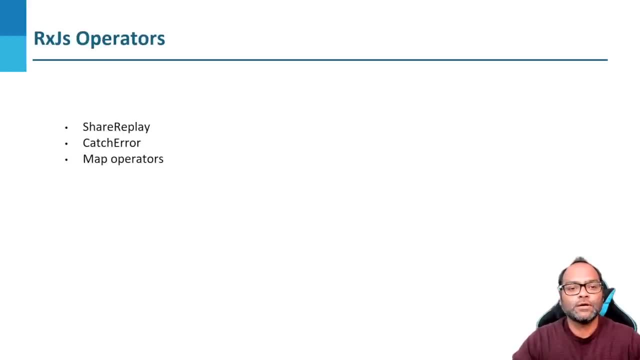 see different types of subject which exist and probably we will move this code outside. so this is it from catcher and so far we have seen two operators share- replay and catcher- and we also saw an example how you can use a sync pipe, which is really great. you should focus more on using a sync pipe as much. 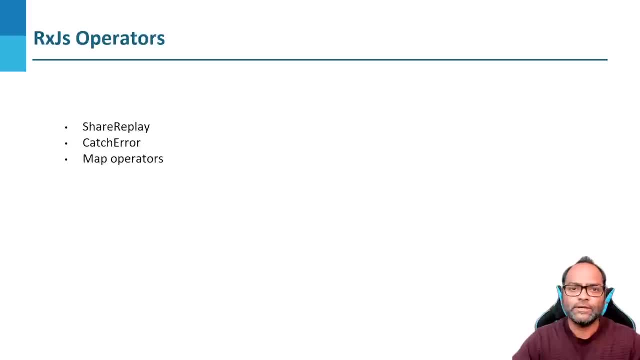 as possible. let's now see an example of map operator. we are going to see some uh, other map operator as well, because there are there are few different, like uh, you will find there is switch map, merge map and uh, there are a few operators like that. so, but here we are going to just talk about. 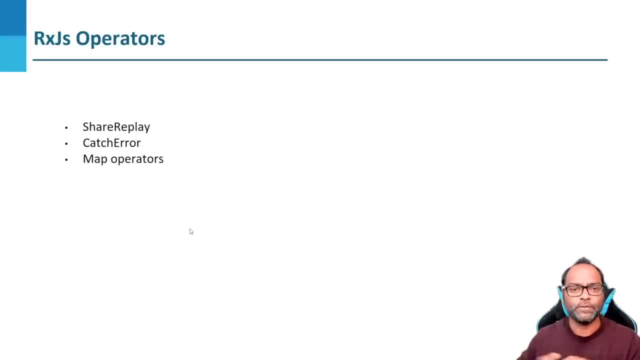 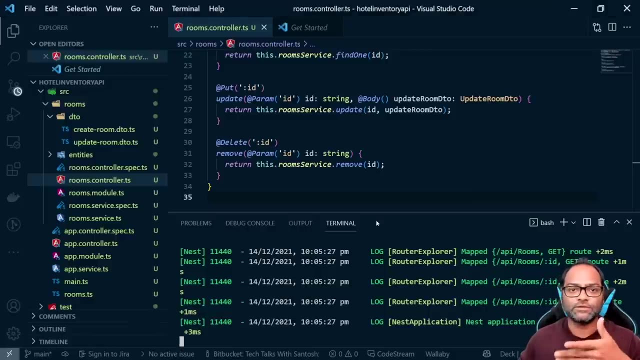 map operator. so let's put in c, see how we can actually use map operator to work with our stream and modified. and, by the way, this is the first operator which we are going to use which can modify, which will modify the data. right, this is the first operator which we are going to use which will modify the data. so far we have seen. 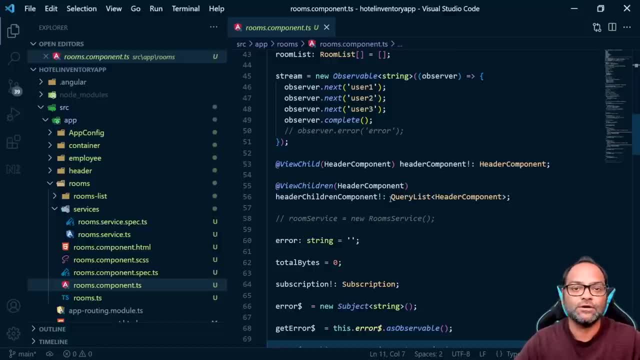 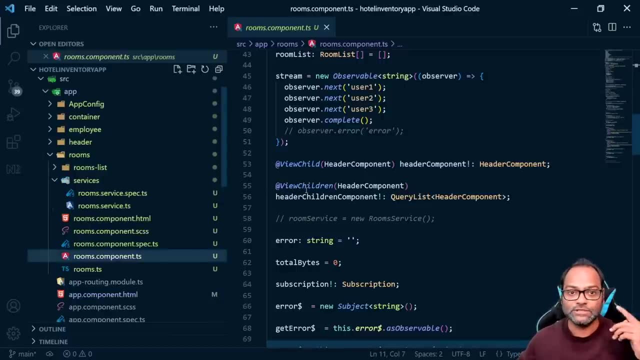 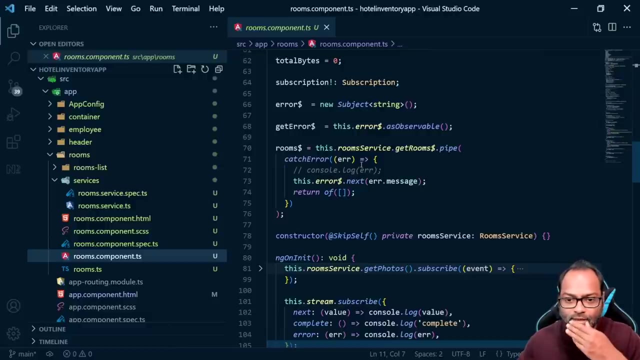 catcher, which was able to catch the error. and we saw- we saw share replay, which was able to cache the data right. so let's see, uh, how we can modify the stream by using share play- no, sorry, by using uh. how we can modify the stream by using map operator. and to do that, what i'm going to do is i'm going to subscribe to the. 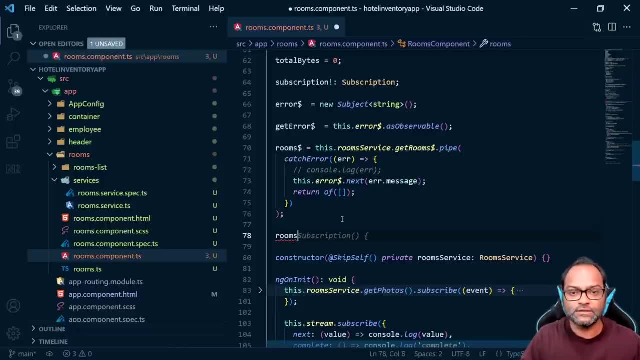 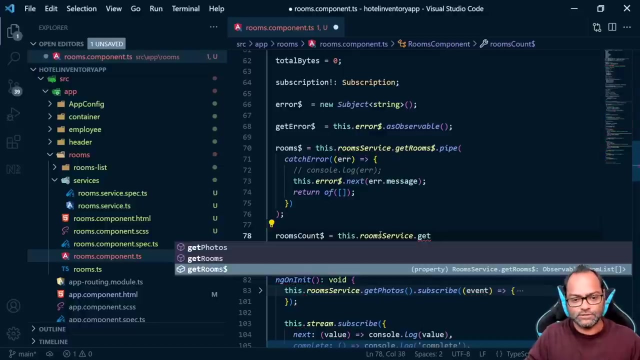 same streams. okay, and i just call this as room account and i'm saying: okay, this is a stream and here i'm going to subscribe. so i'll say this: dot room, sorry, room service, dot get rooms. so this is our stream and then we can use pipe. 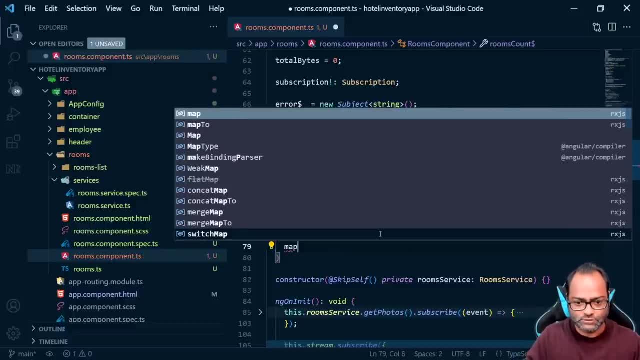 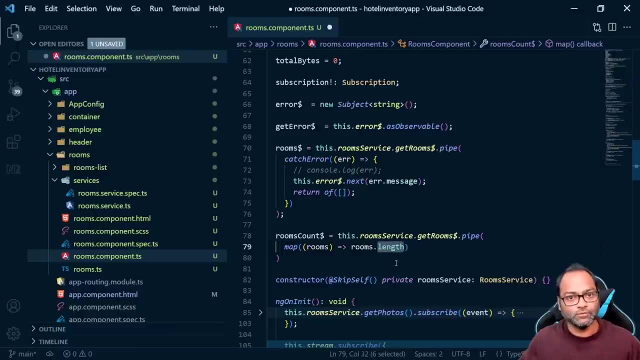 and now in map, using map operator. so we'll just use map and okay, this is coming from rxjs. we'll say rooms and we will take the number of rooms which is available inside this. and now, if you see this type, the important thing is here it is array of rooms and here it is count, which means number of rooms which are available. 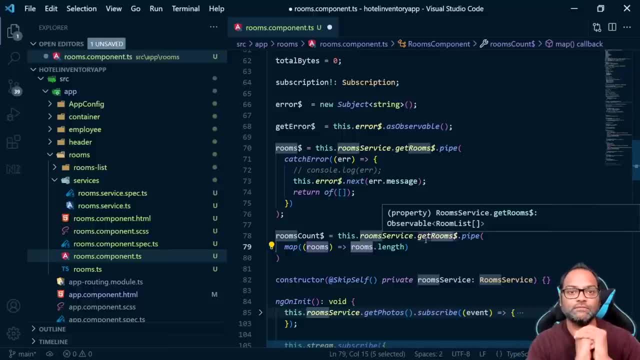 inside this particular array. so we are actually modifying the stream and we are just returning the number of records. or you can see roomslength, which is number of records, number of rooms which is available in this particular stream. but we are not subscribing it manually, we are still. 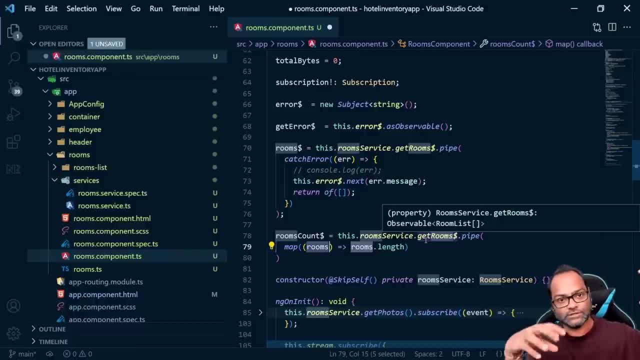 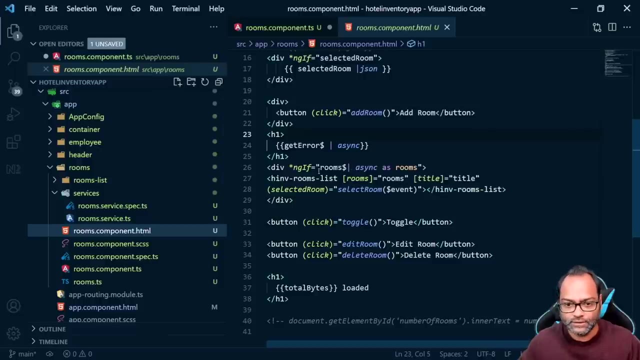 in the stream. we modified the stream and said, okay, it was like room, room of numbers which was coming inside the pipe, and then we took only the count as and we gave that count as a stream. so here now i can just go ahead and use this in our template and let's put it here. 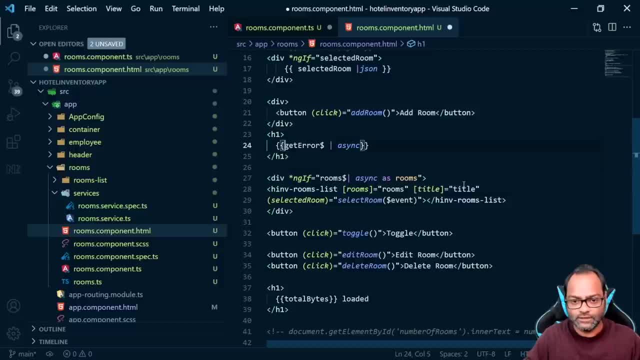 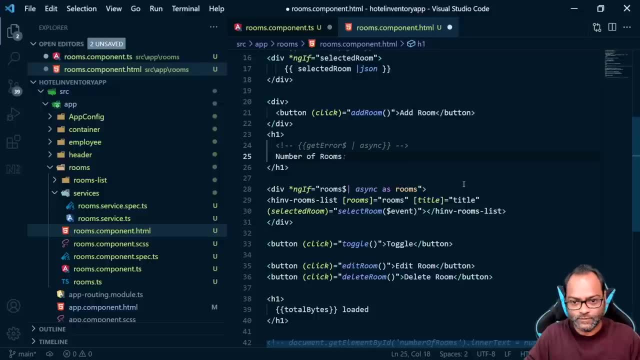 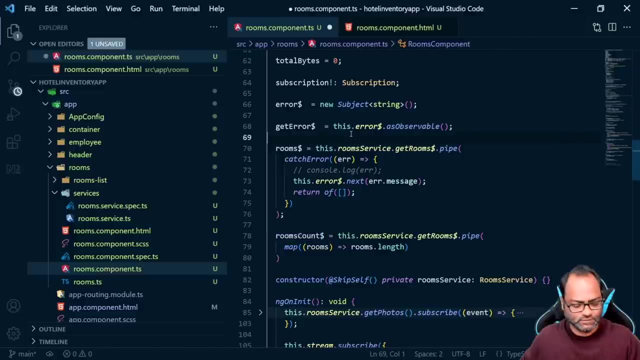 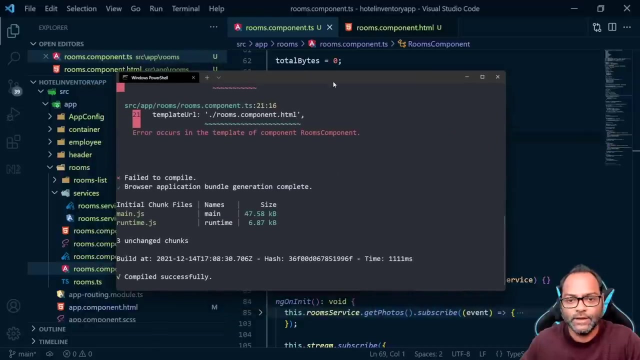 and let's- uh, okay, let's do one thing: let's put it, and it in h1 and we'll see: number of rooms is over sync. and let's save this as well, because otherwise, uh, this variable won't be identified because the file is not saved. let's see if it is compiled. yes, it is compiled. let's go to the. 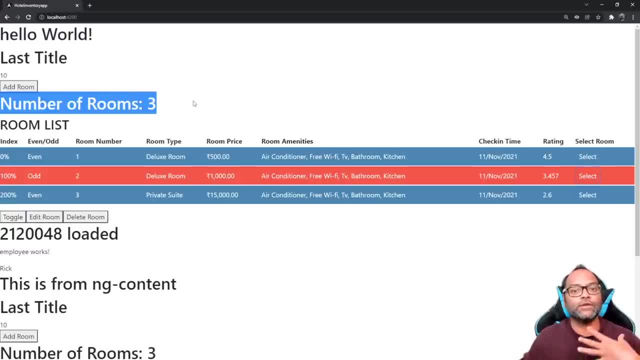 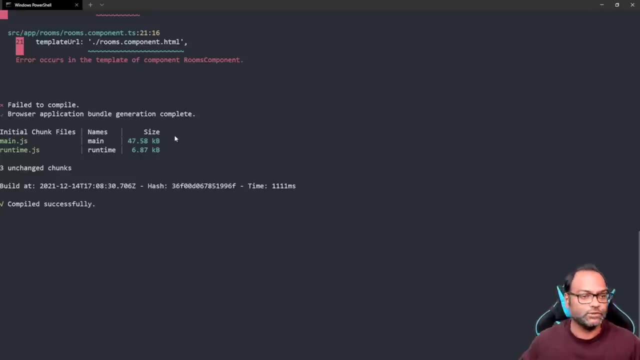 browser and you can see it says number of rooms: three. so this is how you can utilize map operator and uh without subscribing to the stream. you can just get the data whatever you need from the existing stream. so this is uh, the map operator. and now we will move on to the next topic in this video we are going to talk about. 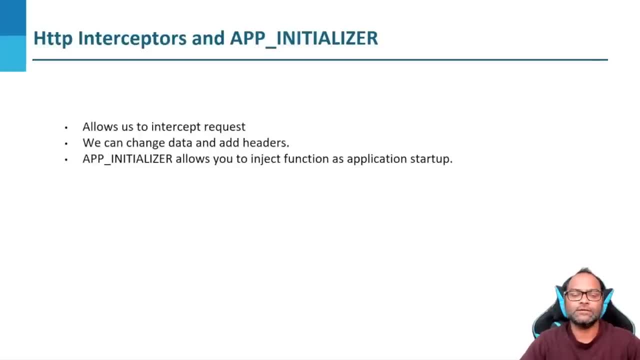 several things. first we will see how we can add the extra headers to our http request, and then we will see how we can actually intercept those requests. that's where the concept of http interceptor will come, and then at the end we will see app initializer. so first let's go ahead and 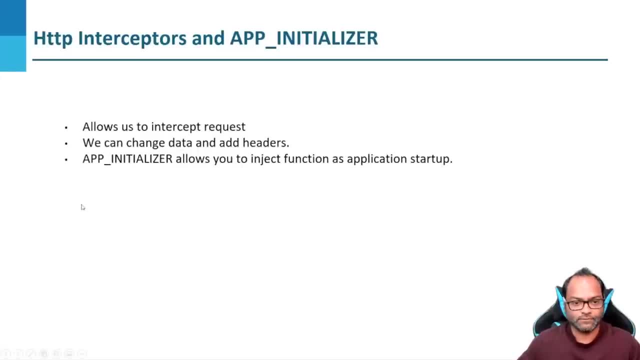 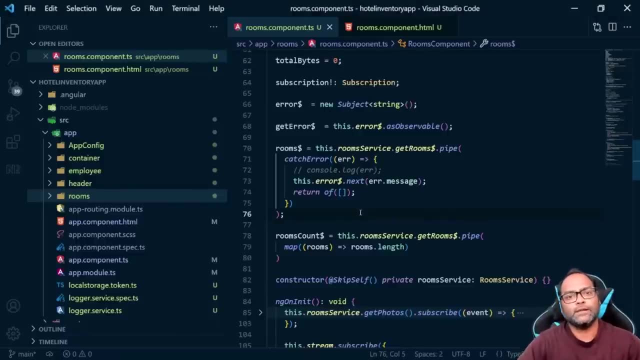 talk about modifying the header information. so we are back to our code base. in your enterprise application, there might be scenarios where you may need to pass some extra information in the header. which header we are talking about? http request header. so we will first learn how to do that. so let's go to our 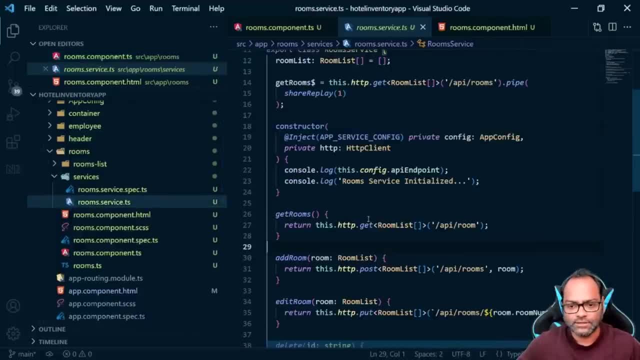 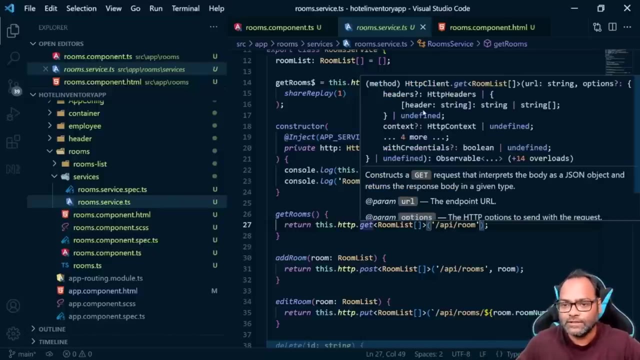 service and let's try to add some extra headers to our. this calls right. so we have get call. we have post call how we can pass that. so if you see the signature of every http request which we have- i mean get post, put everything- you will find that. 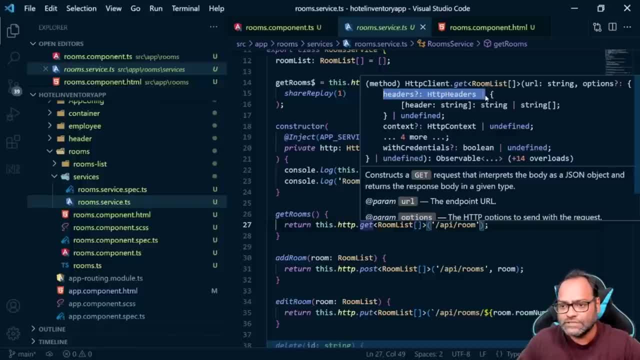 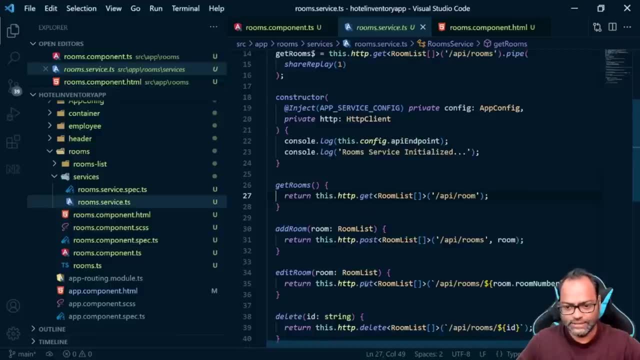 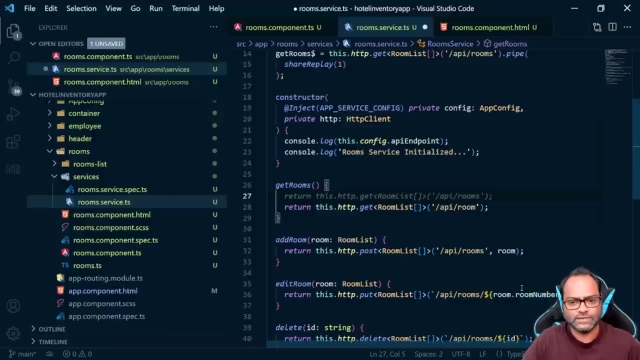 there is something called http headers which we can pass, which takes a key value pair. similarly you will find it for post as well, and post delete everything. so let's see how we can create an http header and then we'll try to pass it. so first let's create the header. i'll call it as: 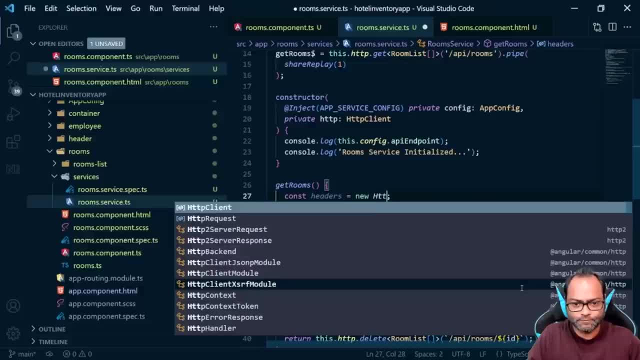 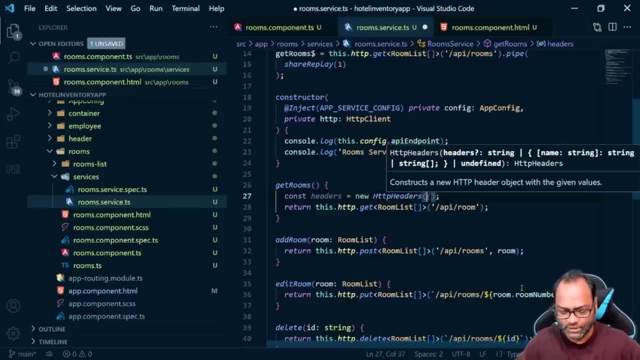 header and it will be new http headers, right, so, uh, as you know, it takes key and value pair. so, uh, few common headers which we see content type you have, let's say, forms, data- no, that's not a header. or you can pass token, right, so token is a common use case. here we are going to pass, let's say: 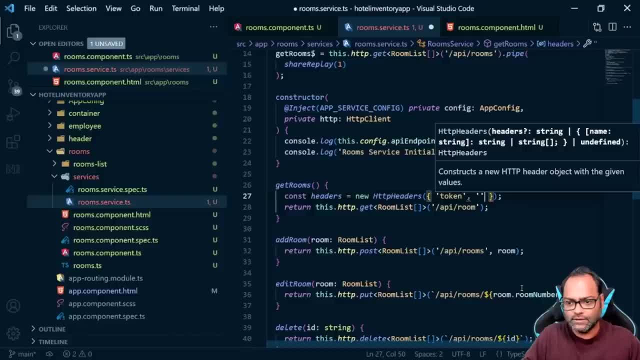 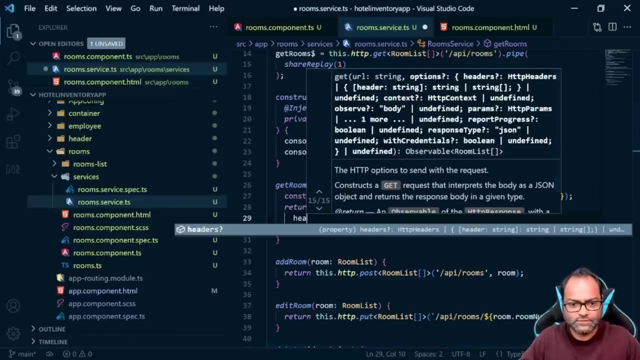 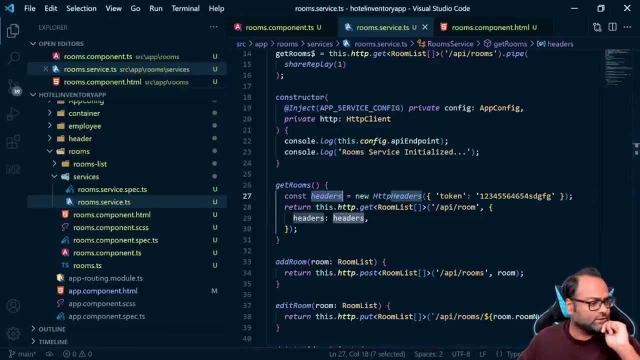 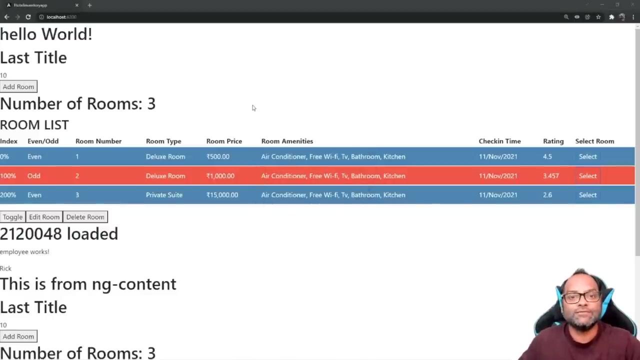 token, for example, and it will take, this is the value. so alphanumeric, let's say our token is some alphanumeric, random value, and then here i can just say: pass this headers to here. so we now let's verify inside our browser that if, if that particular header which we have sent is received or not, 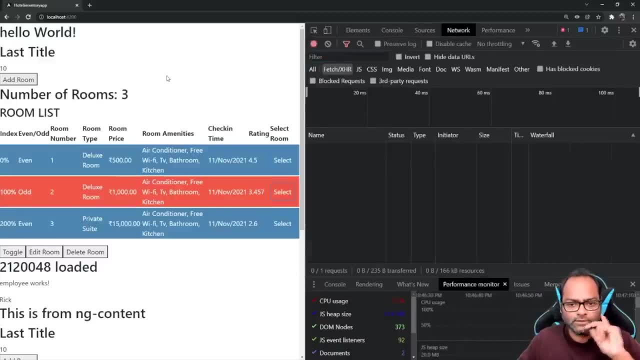 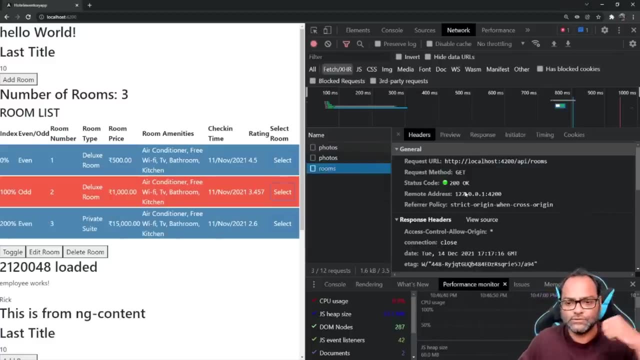 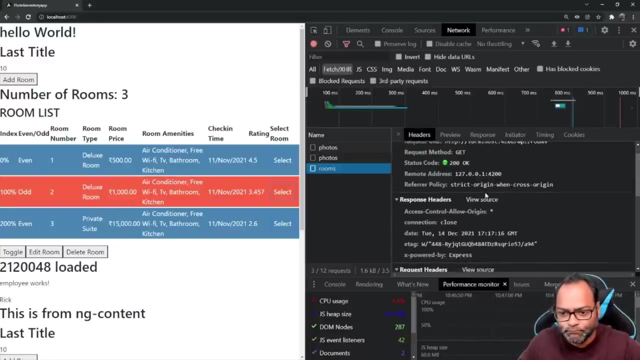 let's go back to our network tab and let's reload this. uh, it's compiled and this is the request which we are trying to see, which we uh, in which we have added that particular header information which is named as token. let's see. so this is response. 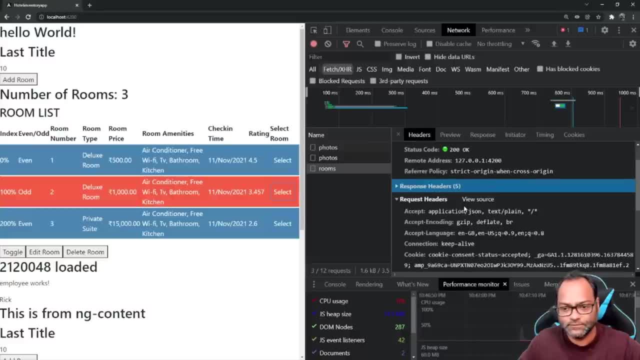 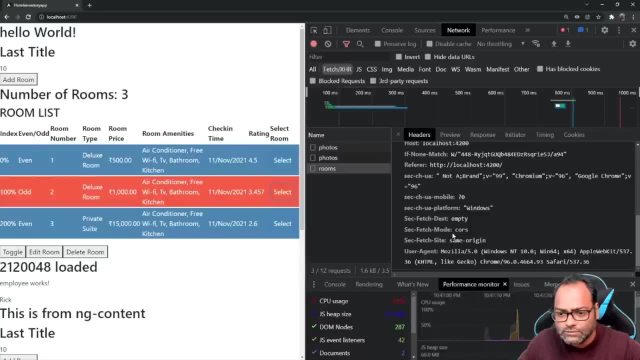 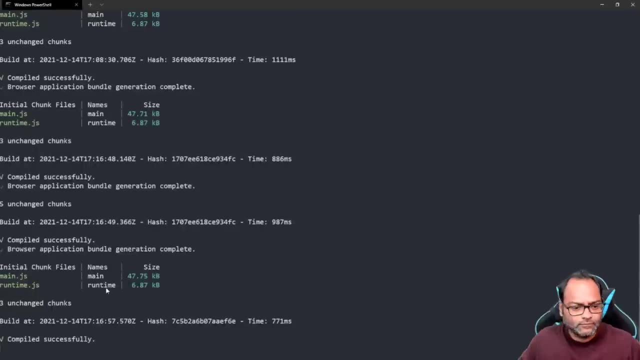 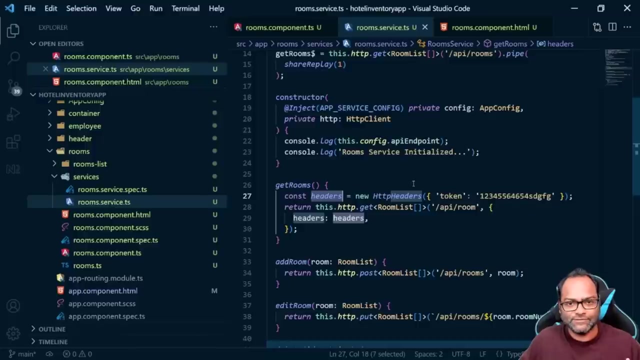 data. this is not what we are looking at. we are looking at a request header and let's see if we have. okay, there is one thing, uh, there's a window, 그는 kimmel. there's a window could be, there can be a window which we have. so, uh, if we're usingotf and then we start to see the escolist 알�vation unique header, we like us to do is, and then we produce this part in the belong historyo and its root of the window and what you can, just place it together and just give it an array of different header. 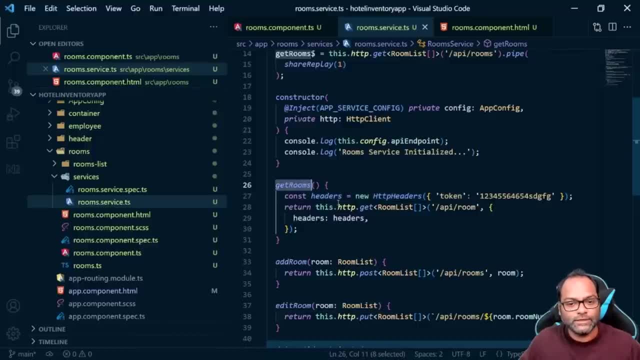 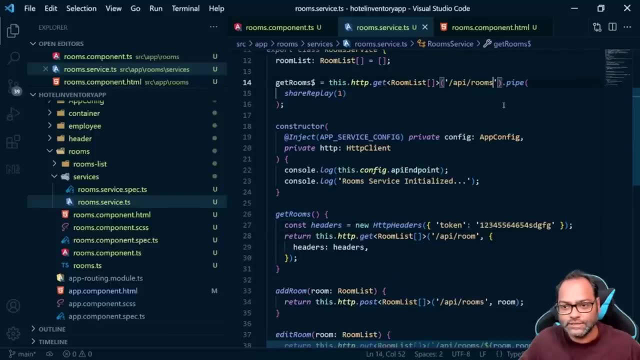 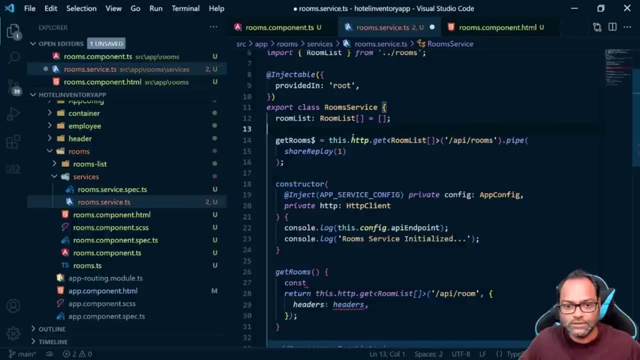 one mistake which I made, if you, I mean, we are not calling this method anymore, so if I have to do this, I have to actually pass the setter information here, right in inside this call. so I'll do one thing: I'll create and cut this and paste it here, and then we'll pass the setter information into. 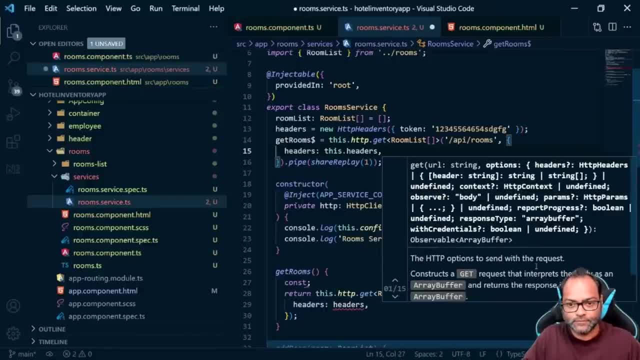 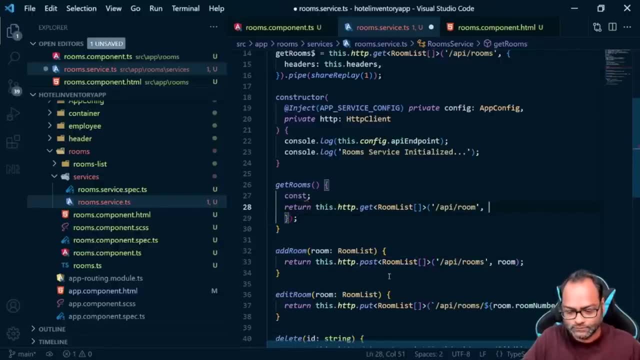 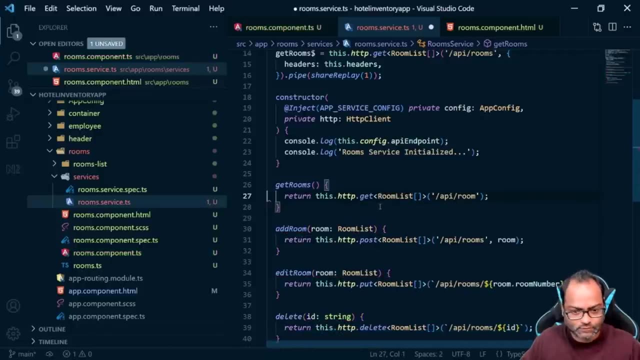 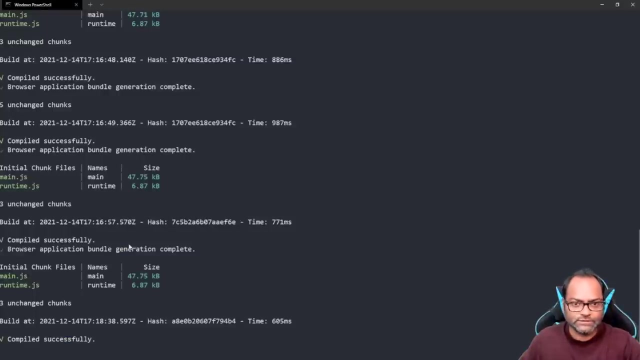 this. just look at us and let's remove it and let's see move this as well. okay, so this is the STD method which we are calling. let's go ahead and verify our build, which is comfort. which is compiled. application is compiled. now let's go back to our code base and let's 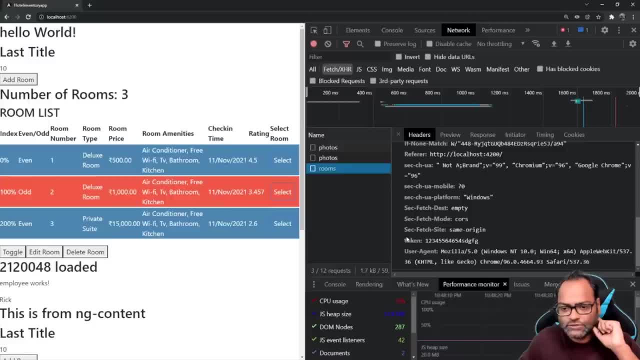 try to see request header now. so we have this token, which is available now. this token can be received from at your api. so, in case, let's say, you are working together with some back-end developer, in it he says: listen, uh, for this particular api call i'm going to need some token. this is the. 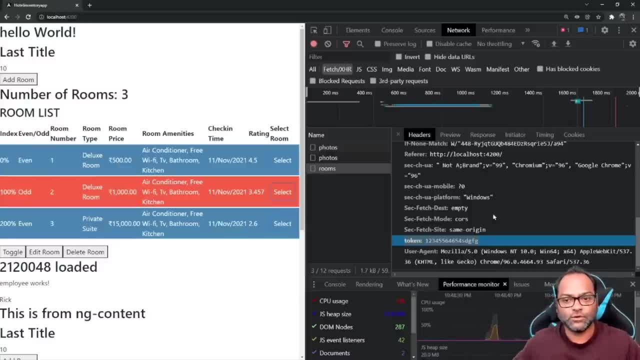 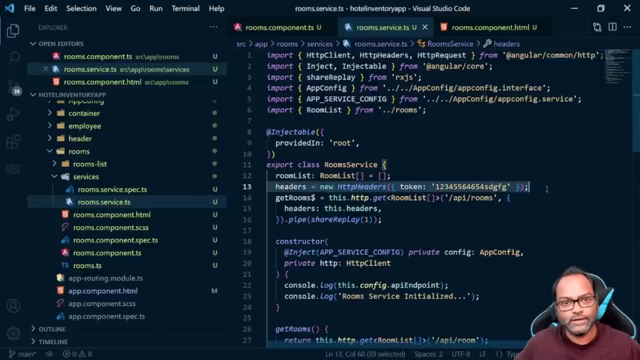 token which you have to pass with every request. so this is this is how you are going to do it. so you will. let's go back to the code and then let's talk about it. so this is how you will create a new header and then you will pass that header into your request. so this dot headers which you 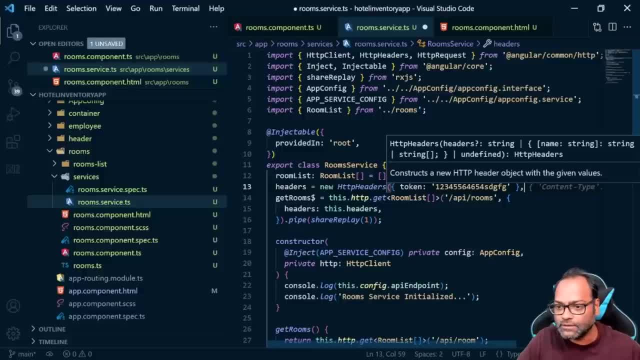 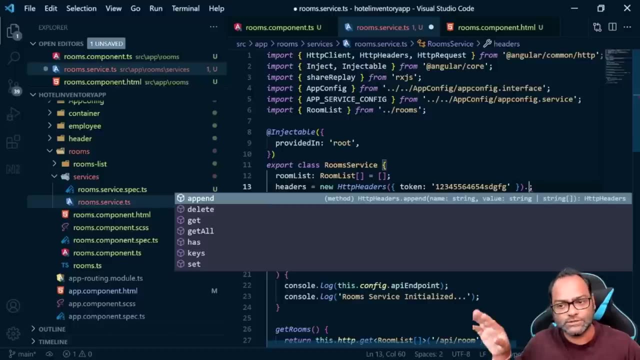 have passed here, and you can of course pass multiple and let's see. so you can call append method and then you can add multiple. so that's how you can do it. you can also see: uh, there is a method to get the headers you have. has has. 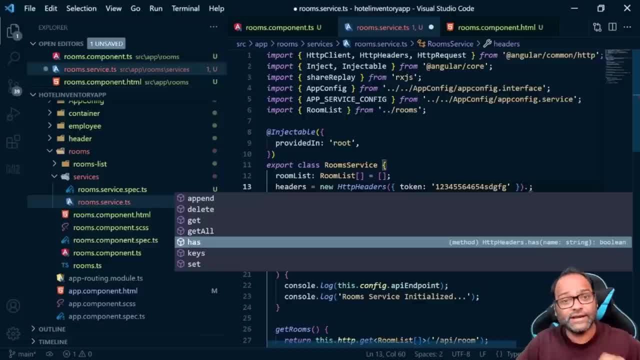 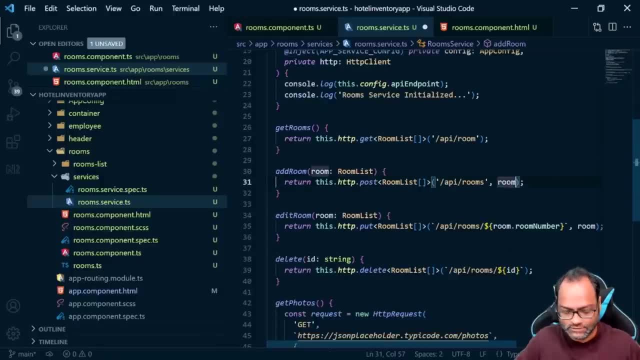 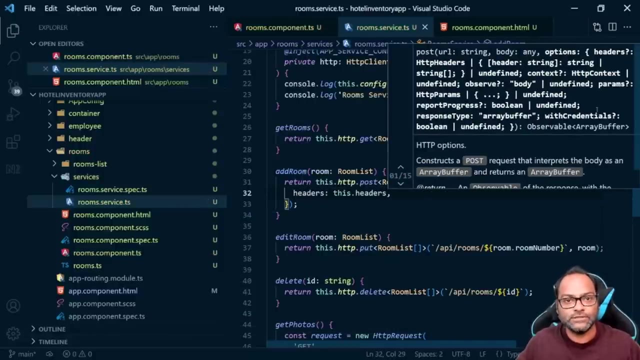 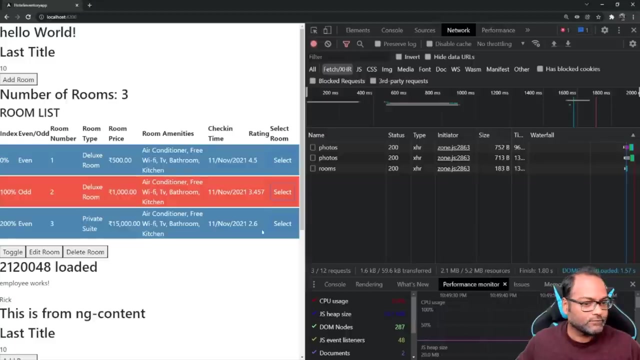 to actually see if this particular header exists or not. so you can just copy the same header. let's say, uh, let's try to add a room and see if it works and we have this information passed or not. so we can pass headers and we will pass this dot headers in add info in add api as well. let's go back to 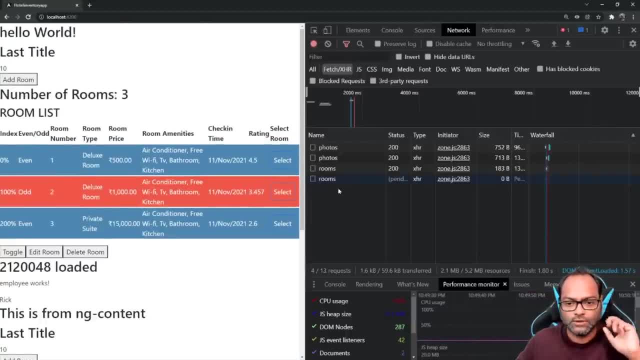 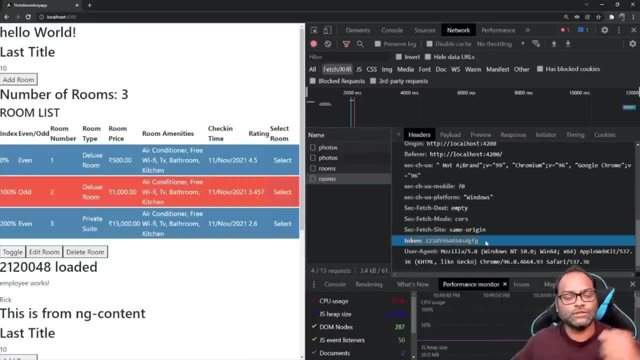 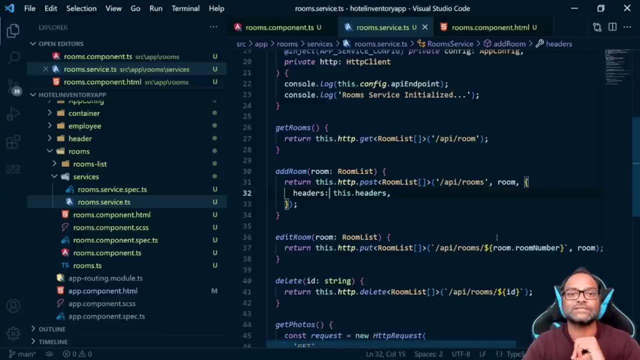 the code and let's add a room, and this is our room, said soon as we will be able to see. token here has right. so this is how you will be adding header information. now, once we know this- how to add header information- let's talk about another use case. so let's say you get it okay, and now the requirement is you have to actually go. 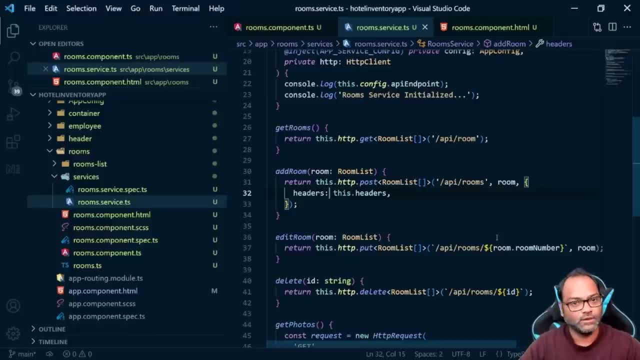 ahead and add this token to every request. do you think the what i'm doing is correct or is the most inefficient way? of course, the answer is no right. i mean, what i'm doing is i'm duplicating the built-in result of the gehen, and what i'm doing is i'm duplicating the built-in. 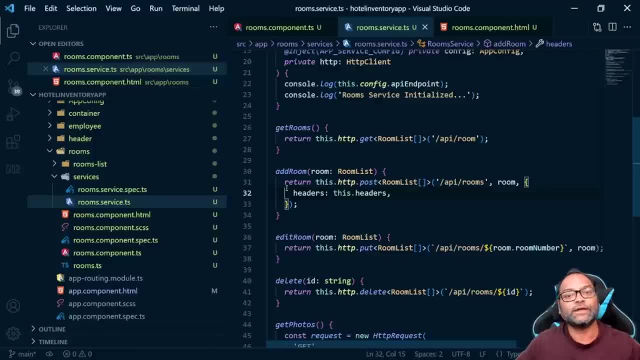 code, which is, of course, I shouldn't be doing that, So what we can do. So this is where the concept of HTTP interceptors come in. HTTP interceptors is not only made for this, but there are bigger use case for HTTP interceptors. HTTP interceptors, I mean, you may have actually. 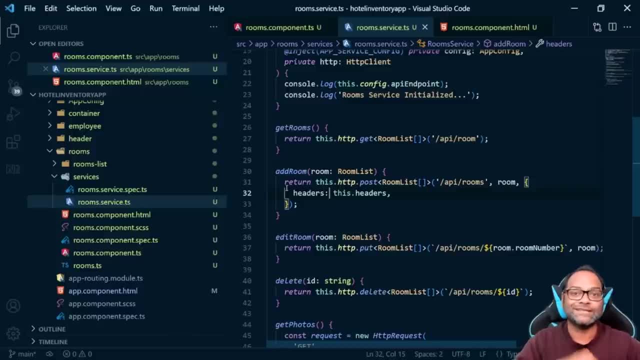 heard about interceptors. Let's come back and talk about interceptors first, before we talk about HTTP interceptors. What do you mean by interceptor? You might have seen some movies right where someone says: okay, your call is being intercepted. What do you mean by that? 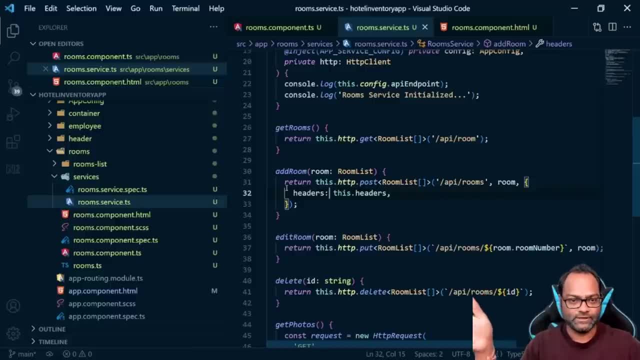 So actually there is sender and receiver, So client is my receiver and server is my sender, right, If you see? I mean, your server is responding to each and every request, right? And your client is also making a request too. So it goes from your client to server and server. 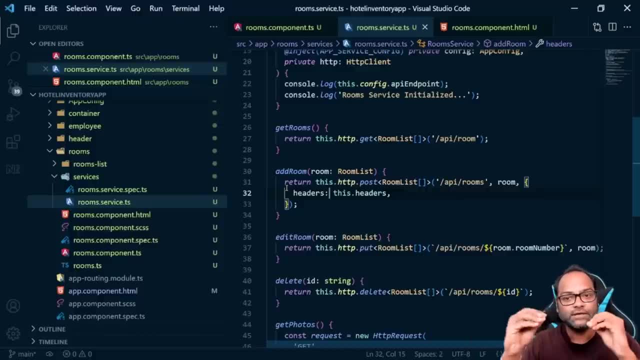 to client. Now there is someone in between who is literally listening to what is happening, what data is going, what data is coming. That is interceptor. So, similar way, HTTP interceptor is a service which will sit between your HTTP call, which is: 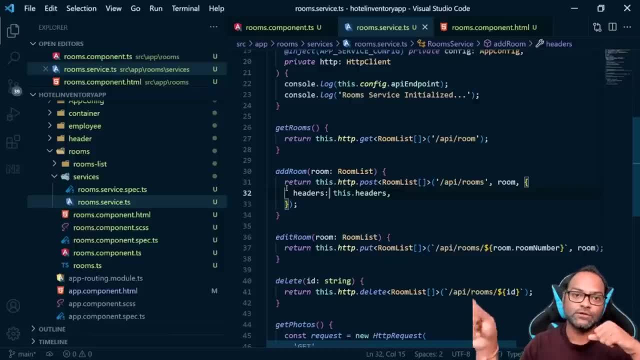 being made from your client, which is your browser to the server, And in case also your server responds, it can also listen to your request. That's HTTP interceptor here. What can be the use case? I mean, there are a lot of things which you can see or do using HTTP interceptor. 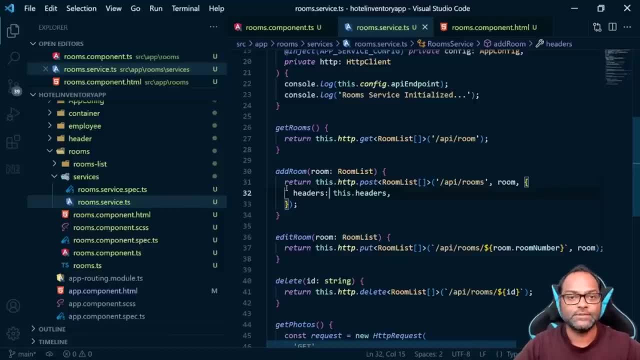 One is, of course, you can add this combinator inside interceptor, so you don't have to add it everywhere. What, what else, What other use cases can be? In case you want to, let's say, add the timestamp to each and every request, Yeah, that's, you can do that. You can do using HTTP. 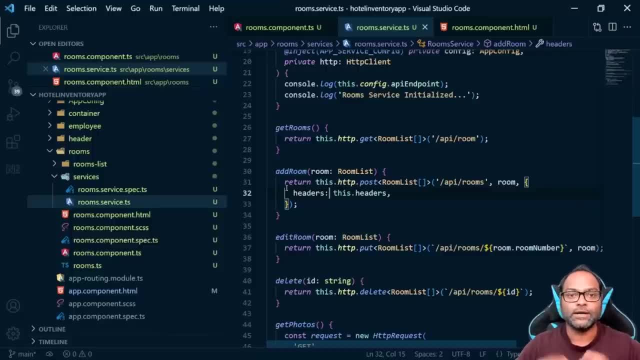 interceptor. What else? Let's say you want to handle the scenario where your token is expired? Yes, HTTP interceptor is the way to go, And you can add multiple HTTP interceptor. It's not like you can only add one HTTP interceptor interceptor. the only thing is it will be called in the sequence they are registered. so let's go. 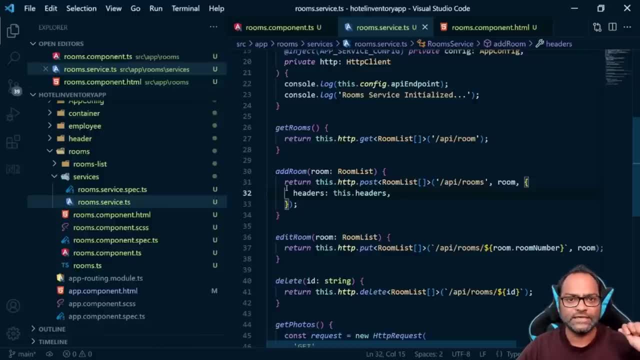 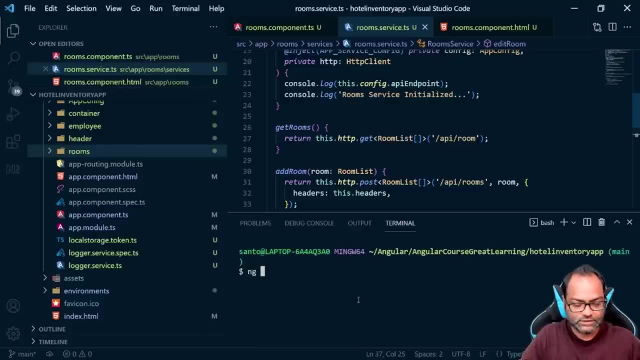 ahead and create our first http interceptor to see how it works, and to do that i'm going to use a command, so, of course, ng g interceptor, and i'm going to call it as let's say, request, request, request interceptor. so, and we have this two, this two classes created and you have this. 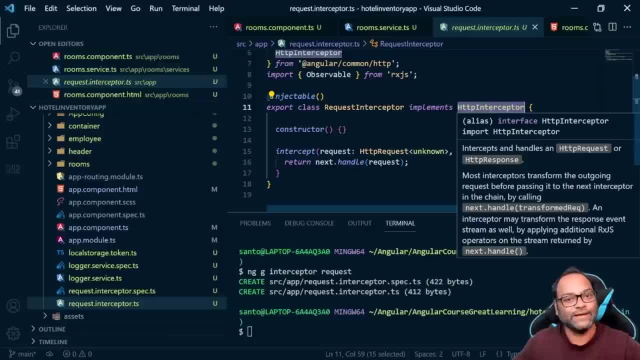 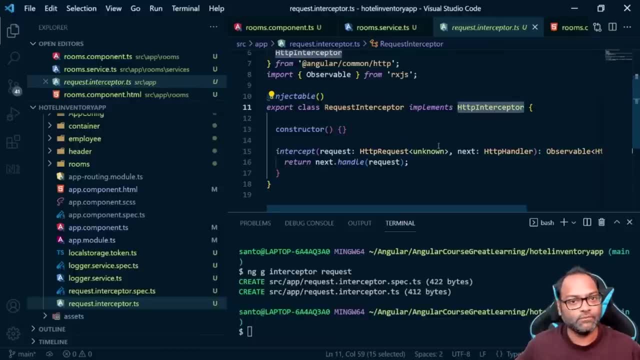 request interceptor, which is which implements http interceptor. that's why it is called http interceptor. remember, http interceptor can modify your request as well, as it can modify your responses as well, in case you want to. now http interceptor has a uh, has actually an function which we need to implement, which is called intercept. 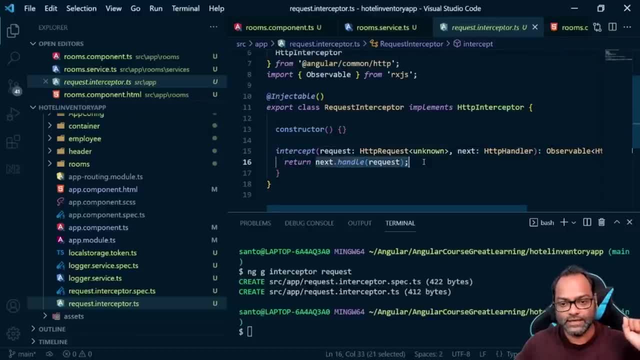 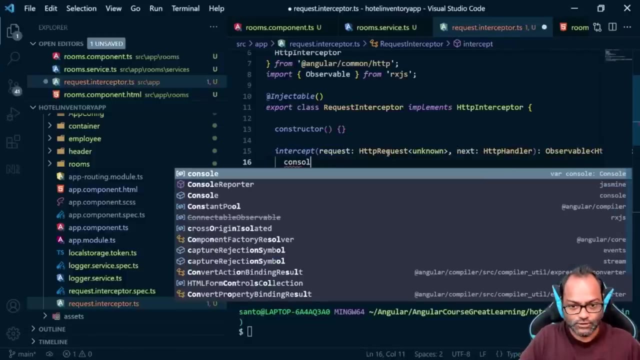 and this is really important- nexthandle. this line actually sends the request to your server. if you don't, if you don't call this method, nothing will happen. so let's try to first do one thing: i'll just do consolelog and we will just log our request. 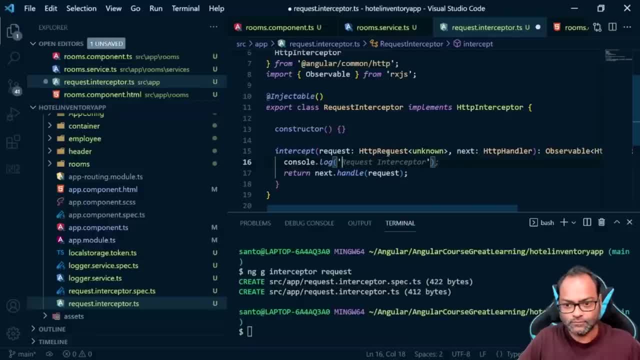 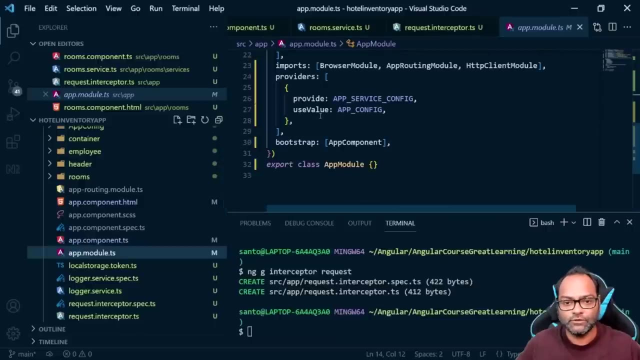 right, so, um, request interceptor, and then we'll pass the request with this. once you're done with this, i mean, uh, right now, this interceptor will not do anything because it is not registered. let's go ahead and register the interceptor. so, uh, we will do it here and 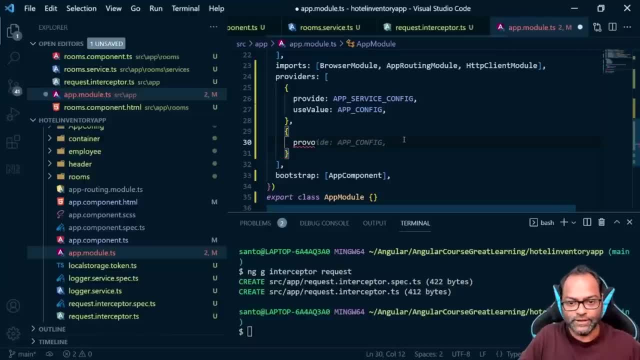 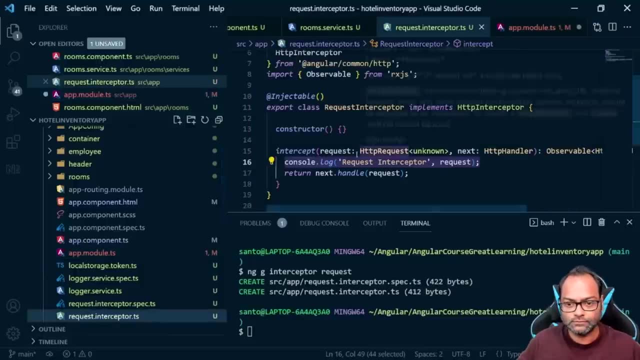 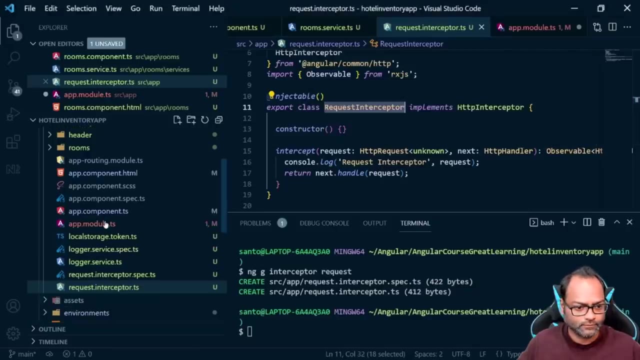 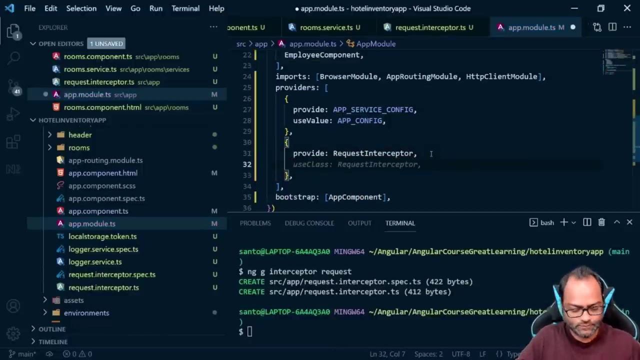 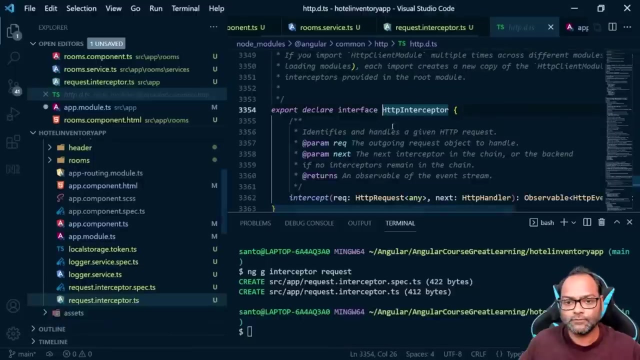 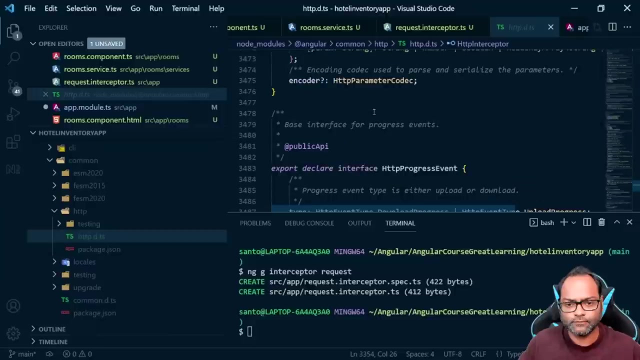 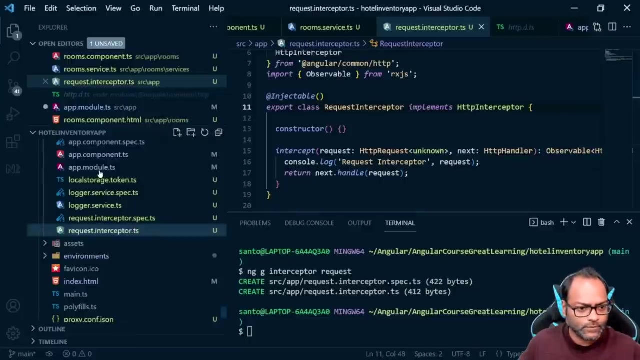 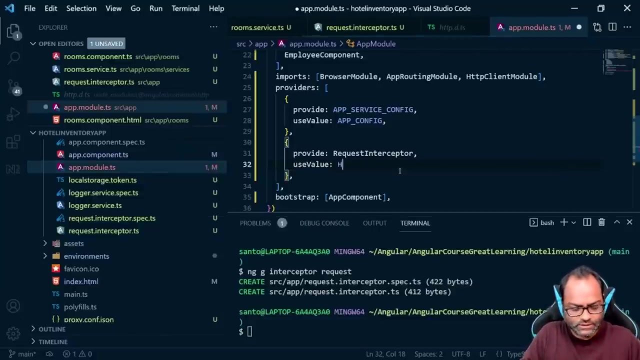 this is the, this is how you you are going to register it. so you will say provide. so we are going to say provide this. so now let's go to the next example, useValue, which will be HTTP interceptors. So let me talk about this. in a little bit of time, we will talk about this, what we are. 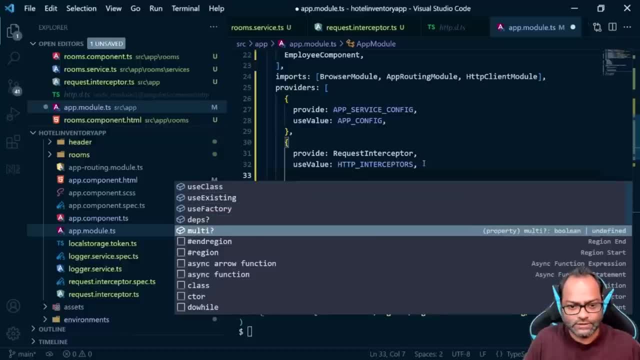 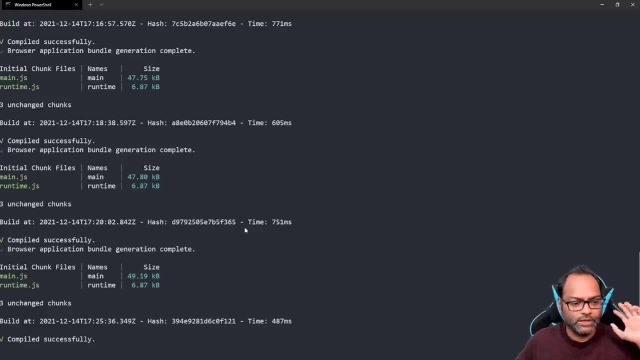 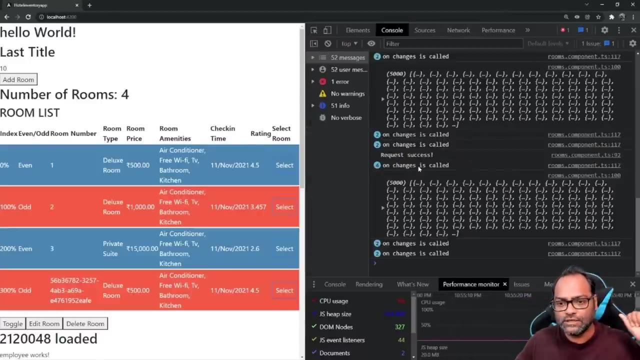 doing here. So we are saying provide useValue this, and then we will say multi true, And let's go ahead and verify first So our build is successful. Let's go back to our application and console, because we want to see the request and request. 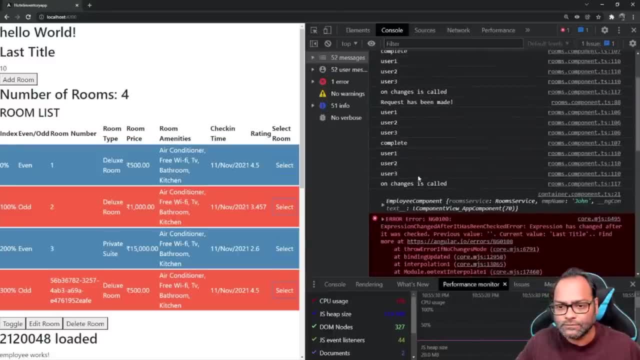 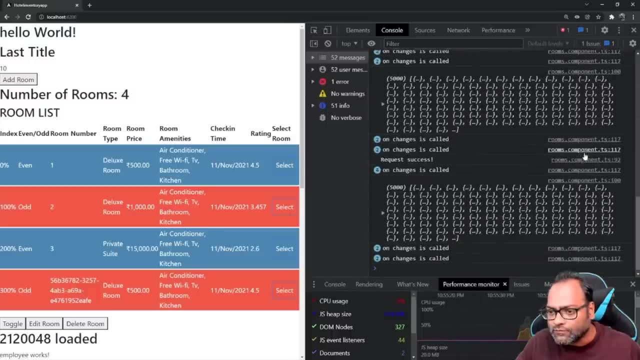 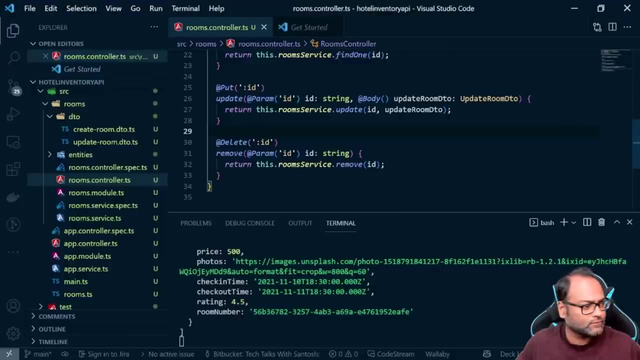 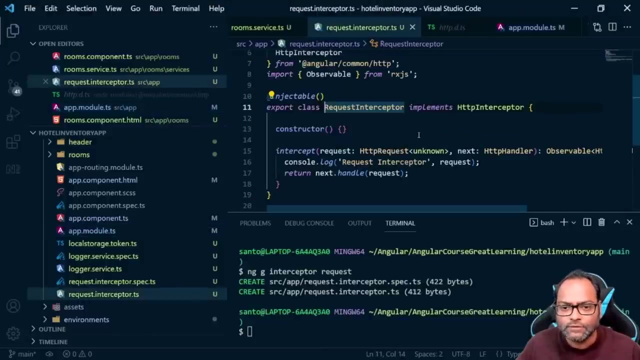 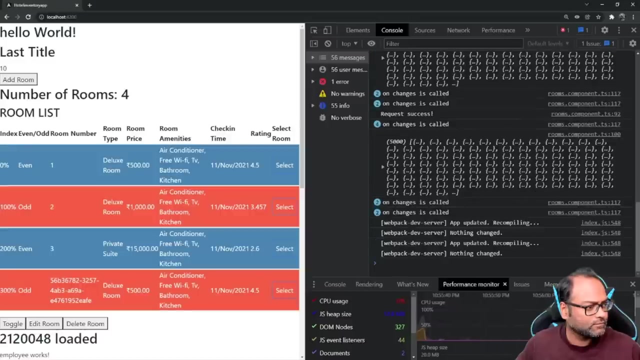 success. request has been made and let's see if there is anything From interceptor. okay, somehow it is not Provide request interceptor, which is our class useValue this multi: true, Let's see our app is getting updated Okay. 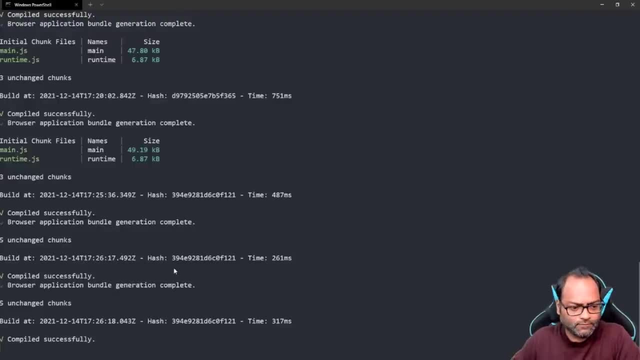 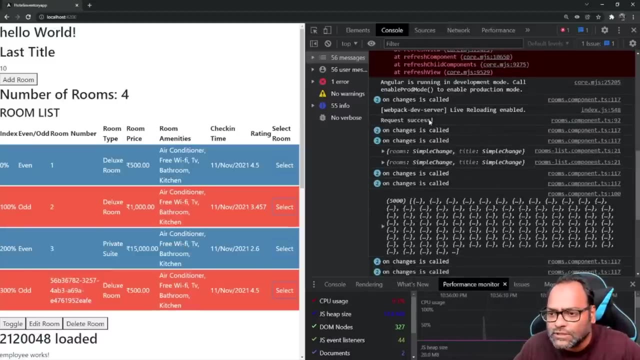 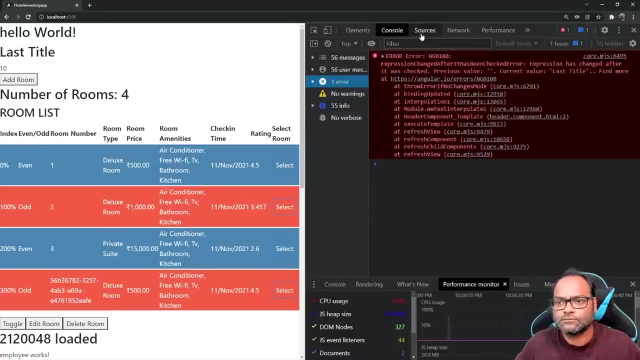 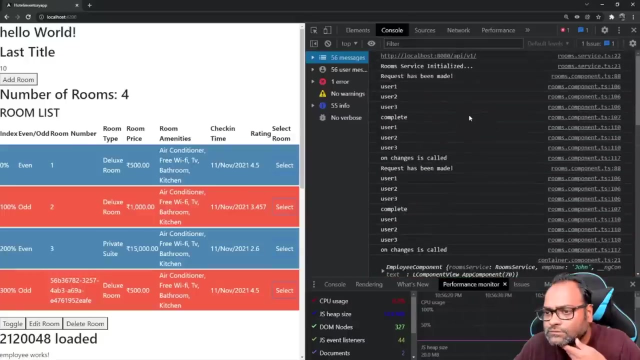 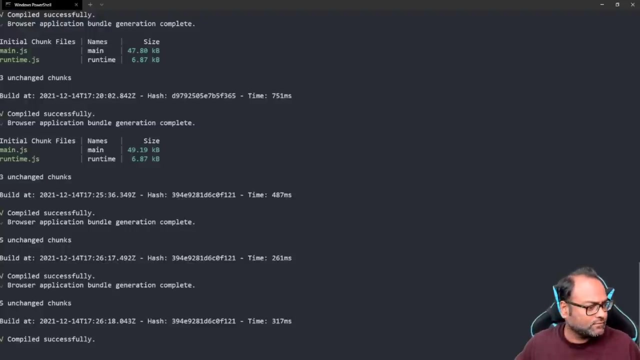 Okay, The build was successful and nothing changed. Okay, Somehow it says: nothing changed. Okay, let's see. Okay, let's go ahead and verify. Okay, Okay, Okay, Let's see if we can see anything. Okay, Okay. 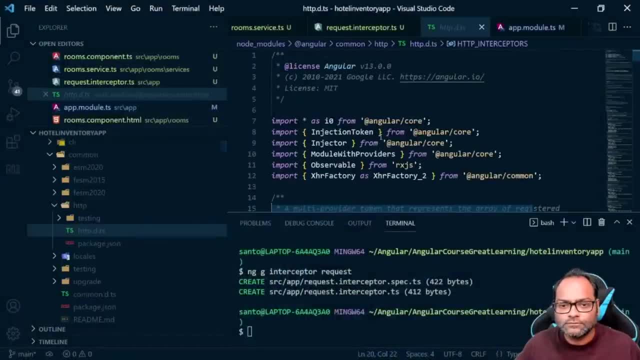 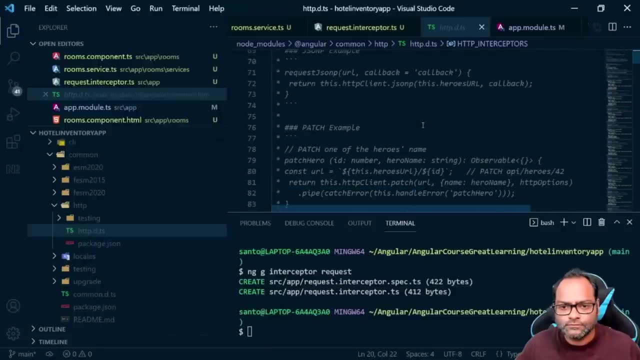 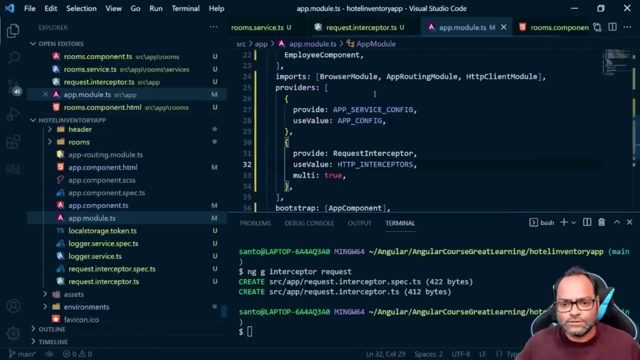 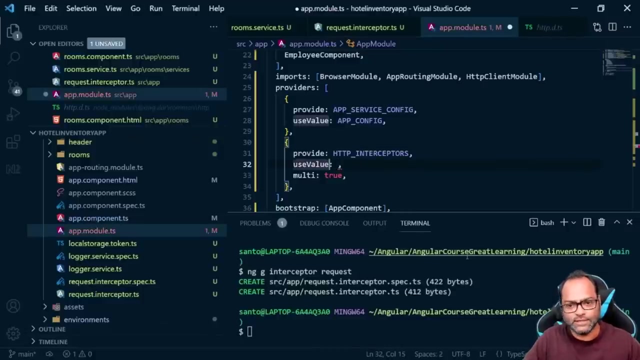 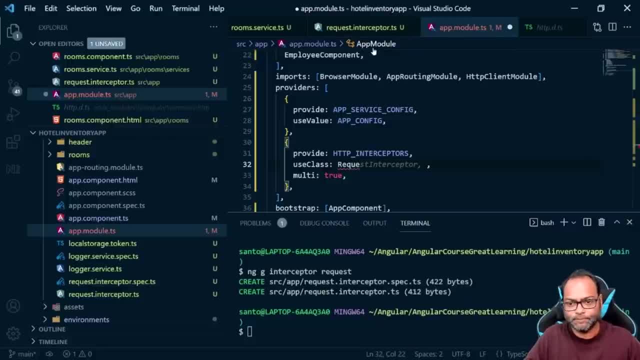 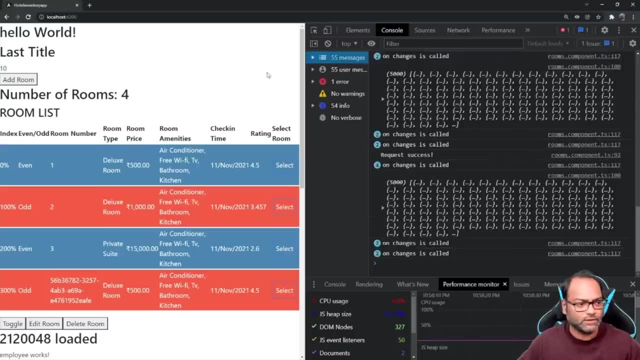 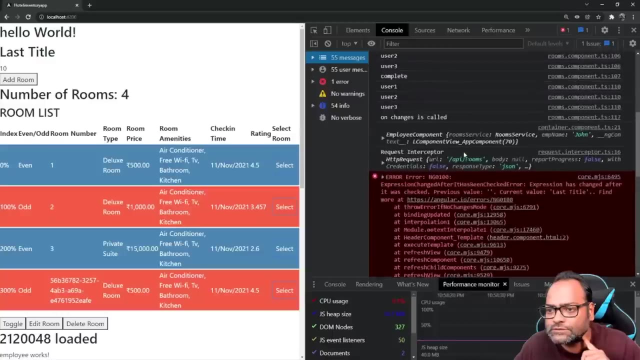 which is our request interceptor. So I just switched the values somehow and let us talk about this and let us verify again in case it is working fine or not, and we will be. we should be able to see now request. here it is, So you can see request interceptor line number 16 and it has everything. 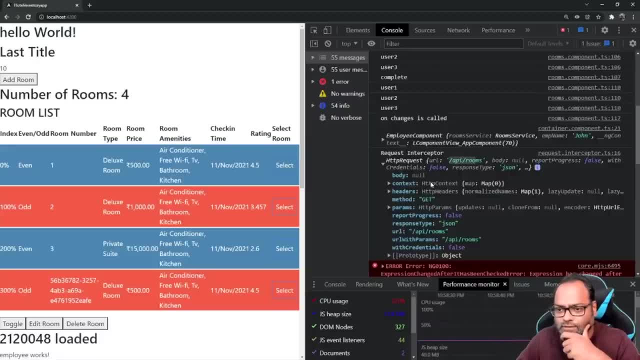 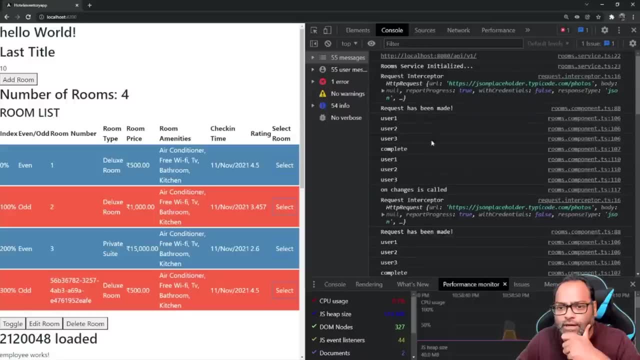 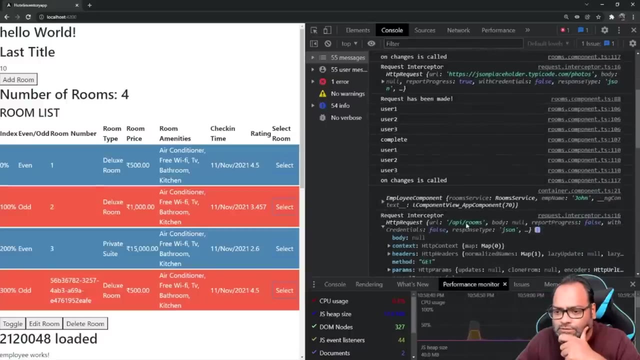 So right now, APS slash rooms is called and we have context body header And there should be one for photos and there should be one for where is the rooms API? This is the rooms one, Right? So you have rooms one and as well as the photos one. 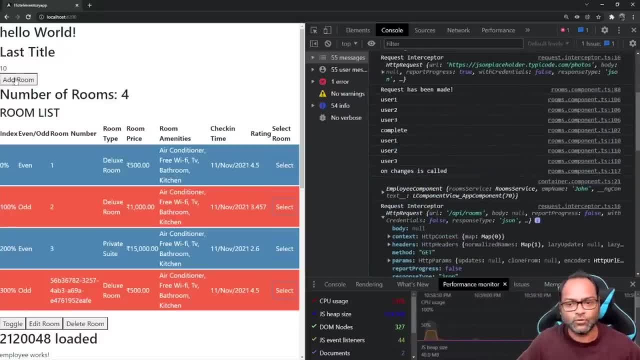 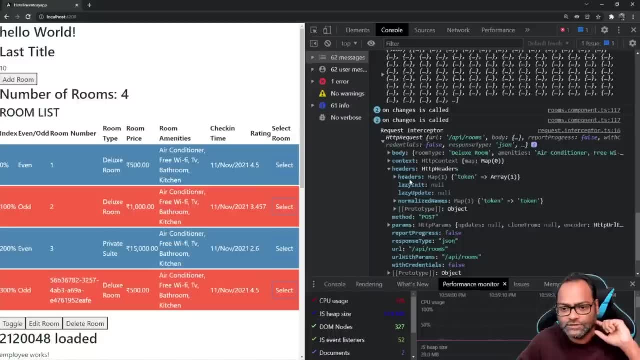 So both the requests are captured here In case we want to add room. you will see when the request is handled here So you can see body context, headers and in headers you will be able to see the token, because right now 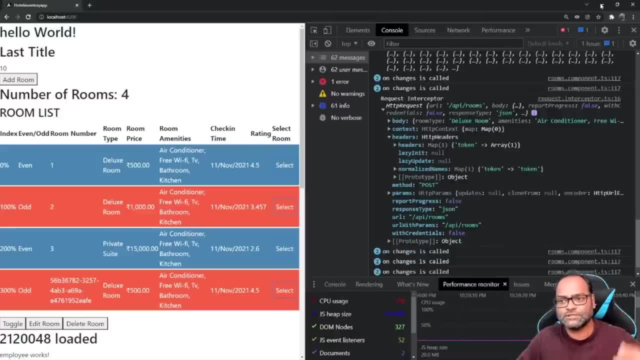 We have. We have one header which is added here, So this is this. These are the information. I mean this. this gives you complete HTTP information, I mean, which is being sent from your client machine to your service server machine. 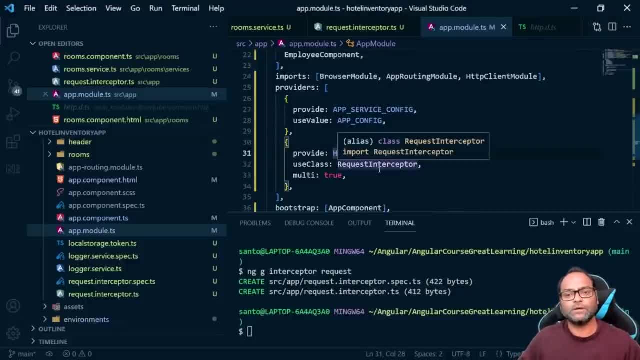 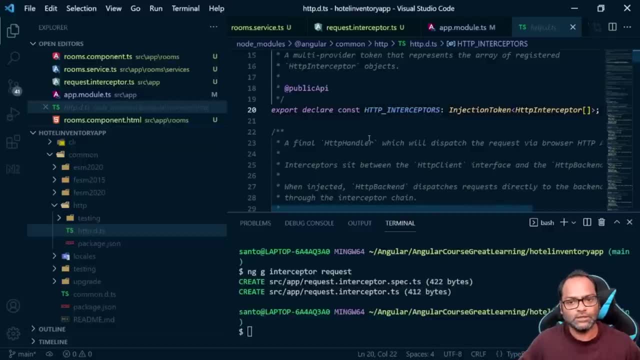 Now let's come back to this and talk about this provide and use class. So here, this HTTP interceptor is nothing but a token. So, remember, we created an injection token and this HTTP interceptor also is also the same. So here what we are saying is we are saying: 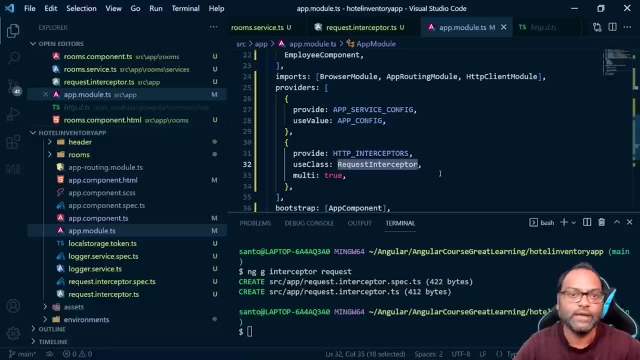 I have created a new HTTP interceptor by implementing the interface HTTP interceptor. Go ahead and add this HTTP interceptor into list of interceptors which already exist, And you might be wondering which interceptor exists? Yes, So Angular internally adds a lot of interceptors. 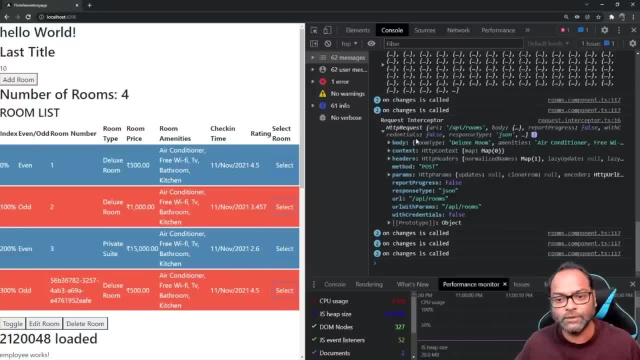 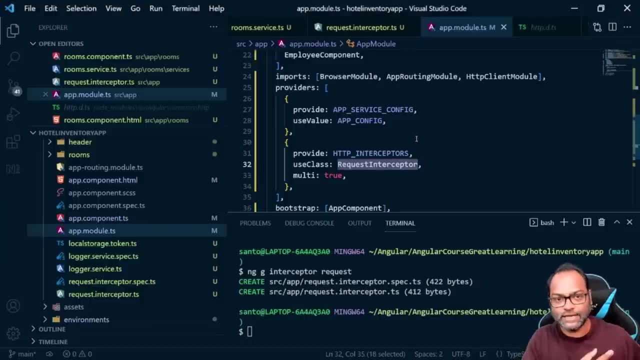 The reason being: if you see this information right now, are we preparing this information? No, we are not. This is something which Angular is doing by itself, So of course it has some list of interceptors which is internally implemented. 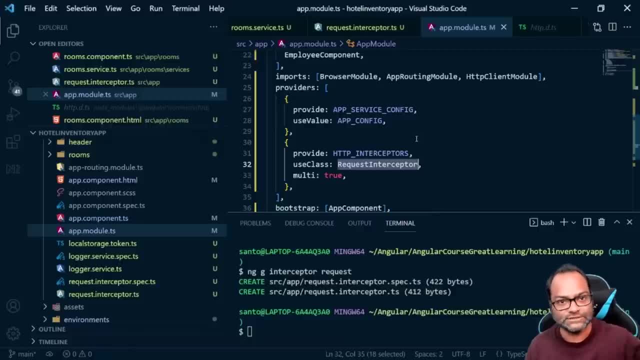 And then we are adding our own. So it will be executed in sequence. So once every interceptor is executed, then this will be executed. If we add one more after this, in that case first this request interceptor will be executed And after that the next interceptor will be executed. 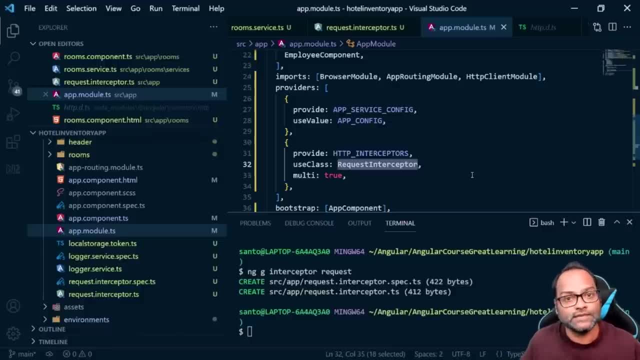 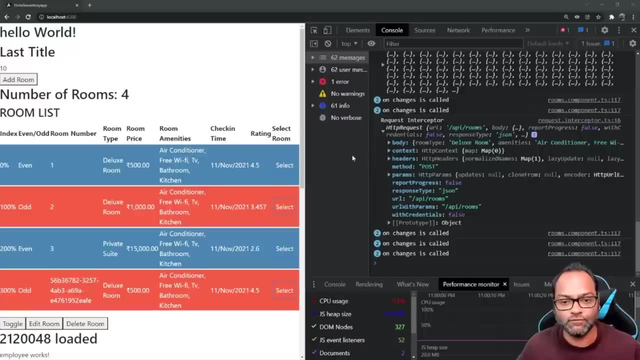 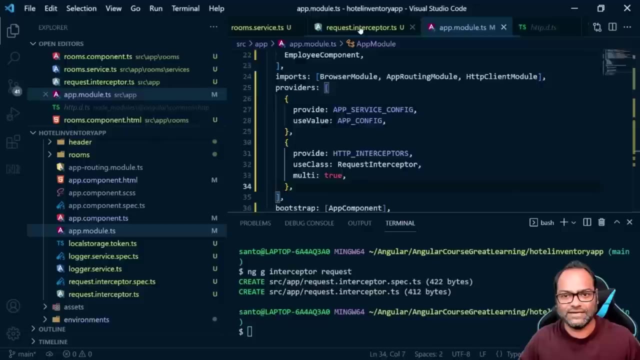 It will always be sequential. Remember that in case you end up adding multiple interceptors, So remember the sequence. Now, here we have the information which is needed, And now we understand what HTTP interceptor does for us. Now let's go ahead and utilize that. 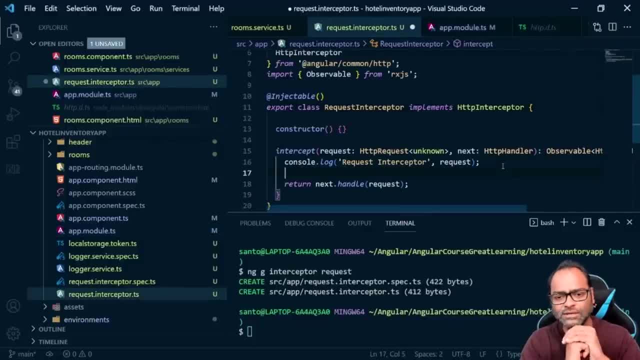 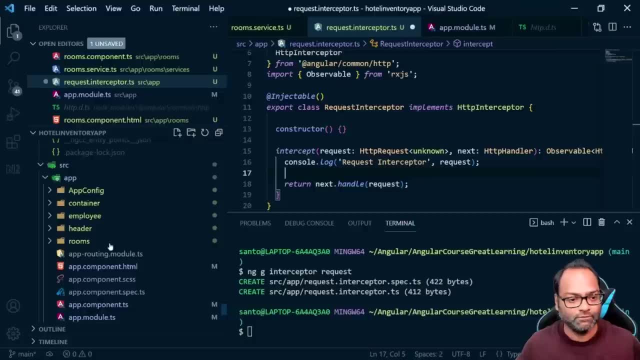 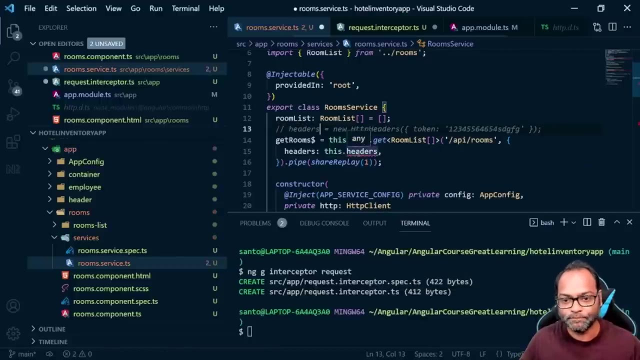 So here what we are going to do is: let's first add the header information. So right now we have added the header information inside the service. We cannot do it for each and every API call, So let's remove it from here. So I'll just comment this out. 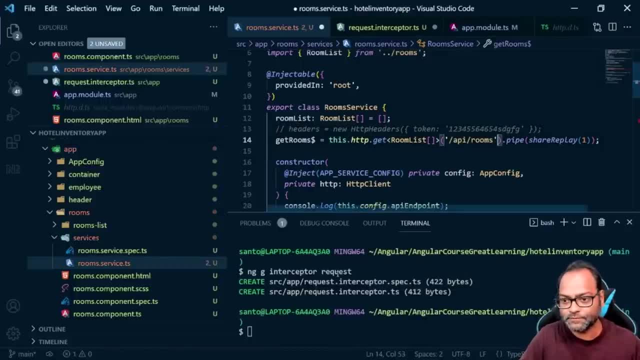 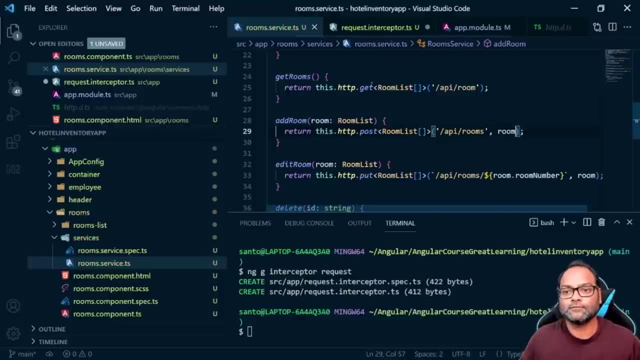 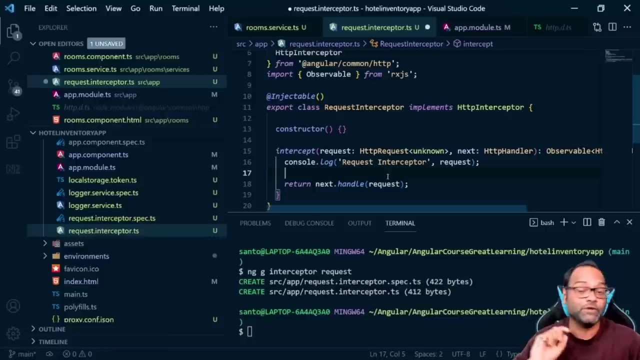 Remove this From here. Similarly, I'll remove from add. And let's come here. So, first thing, you cannot directly modify the request. You cannot modify the original request, So let me just rephrase it, because it may cause confusion. 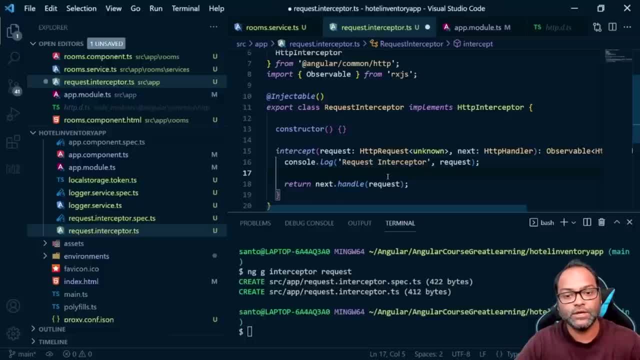 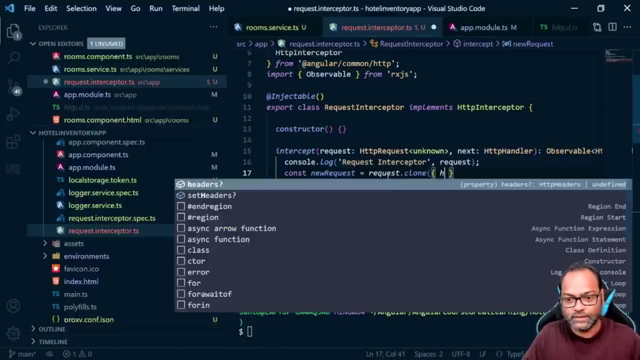 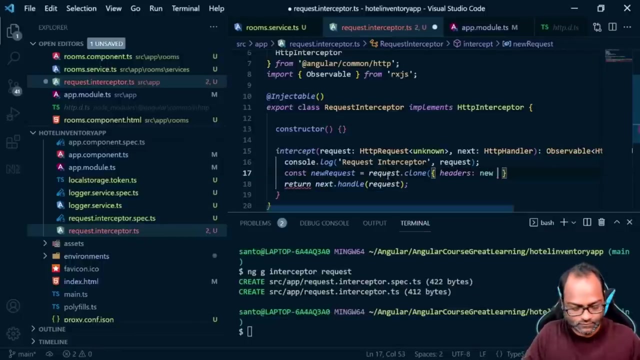 So you cannot modify the original request. You can clone it and then modify. So I'll say: okay, this is new request. Ons Request is equals to, I'll say, requestclone, And here I can pass headers which will be, I'll say, new HTTP headers. 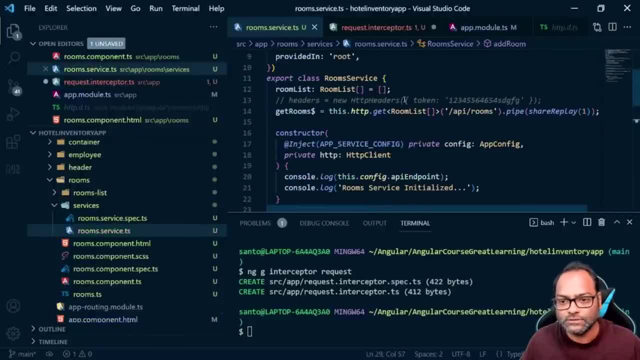 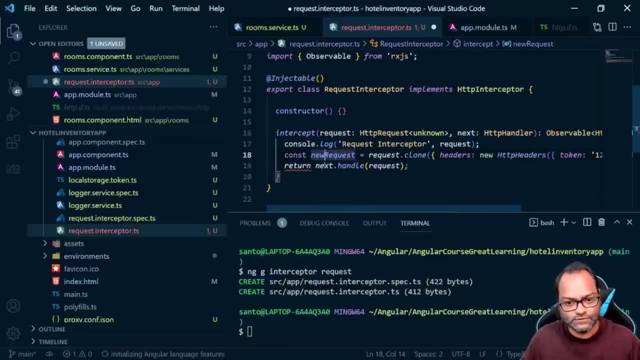 And now let's copy the key and value from here. So I'll say: this is token and this is the value, And the one thing which we have to do is now we have to pass this request, Not the original request. remember that. 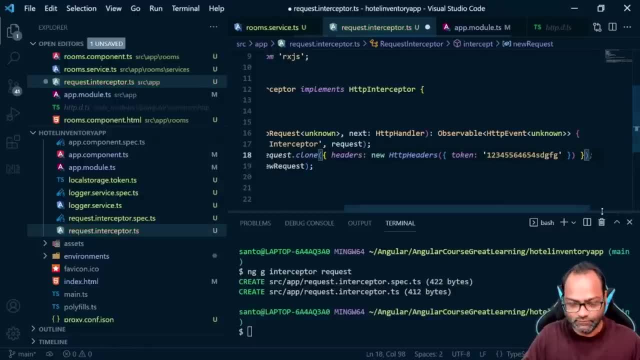 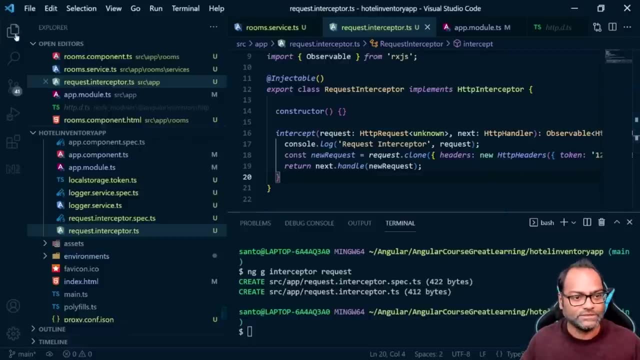 So it happens a lot of times that I end up just passing the same request And then I see, okay, why the modified values are not there. So it's absolutely fine. Everyone makes that mistake, So, and let's format using Prettier. 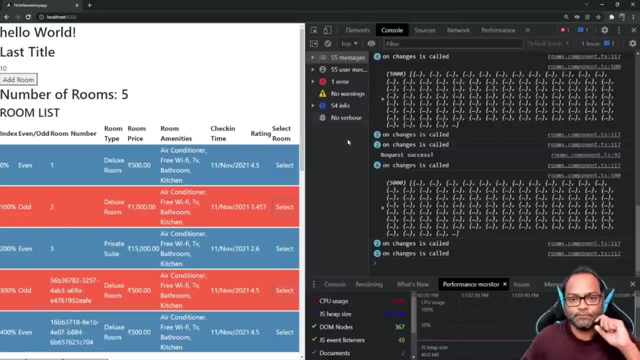 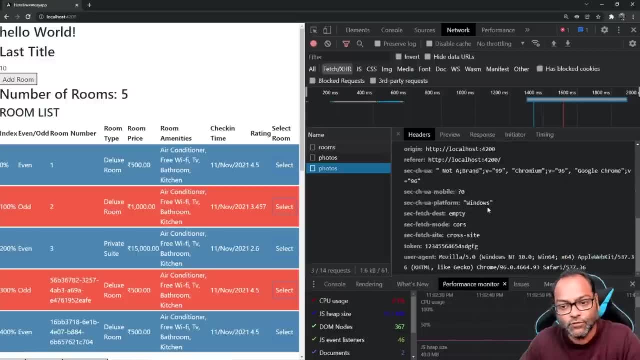 And now let's verify the application again. So we have a network tab. Let's go to photos, And photos should also have this token. So you can see the token is available here. Did we add it to photos? No, we did not. 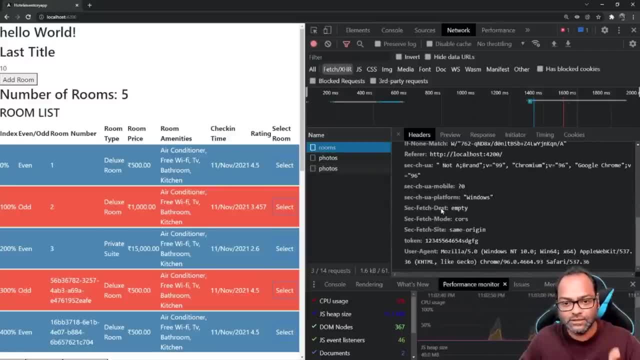 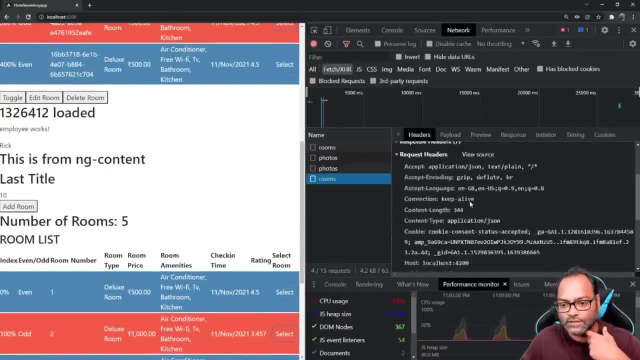 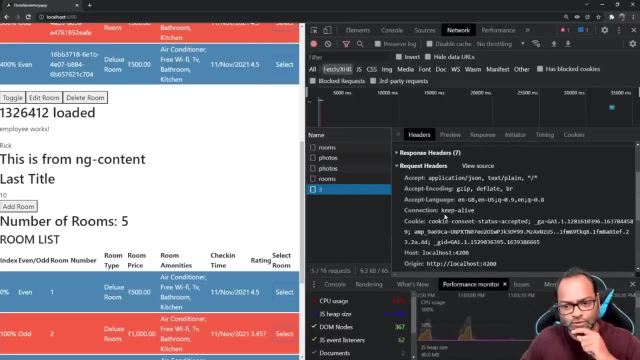 Who is adding it? The interceptor is adding it. Similarly, in the rooms you will find the token available. here You will just: let's add a room and we will find that. okay, it is also added. here. You have inside room. we call delete room and inside delete room also. you will notice. 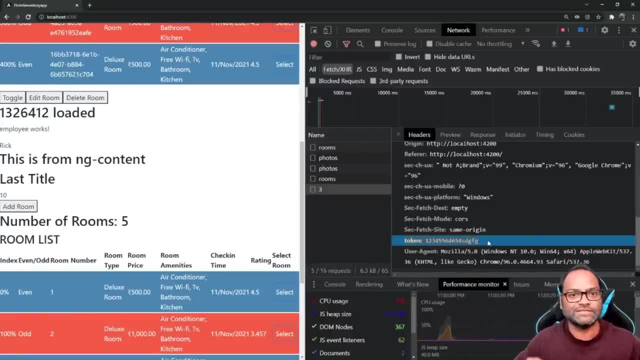 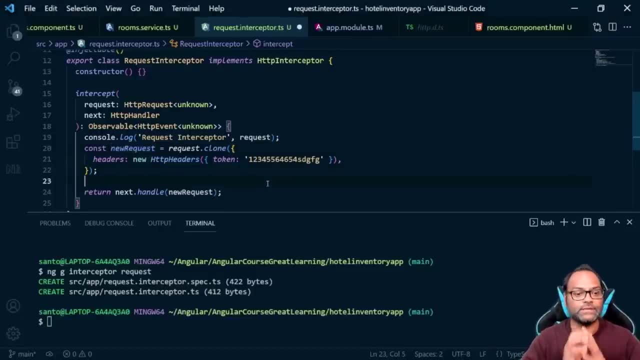 that token is available. So now, with each and every request, the token will be appended. You can add it to the request. You can do, of course, more things, For example, let's say, if you want to handle or you want to create some use cases only. 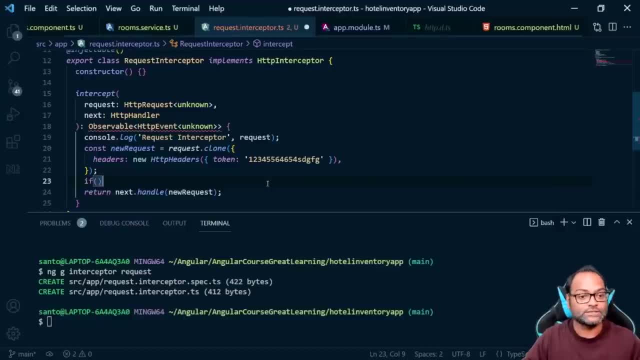 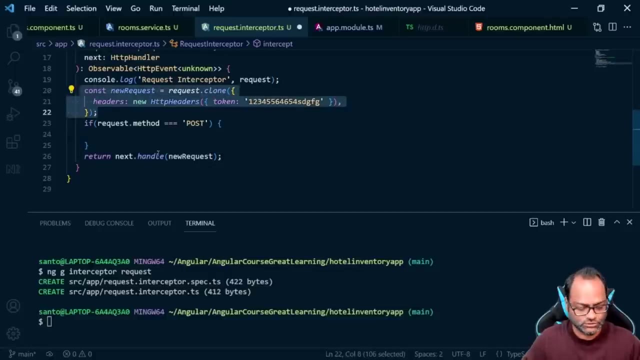 for get request, not for post request. you can do that because this request information. you can see it has a lot of information. So you can say requestmethod and let's do it for post only. We will add this information header: information only for post. 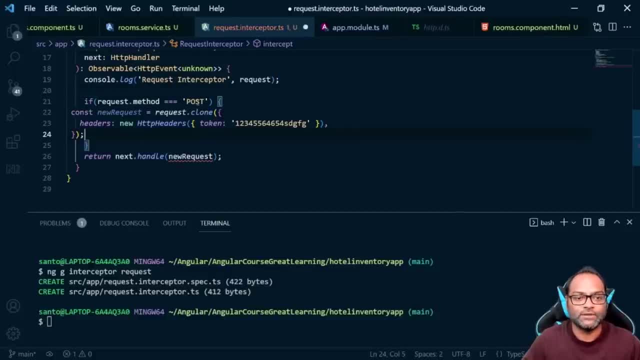 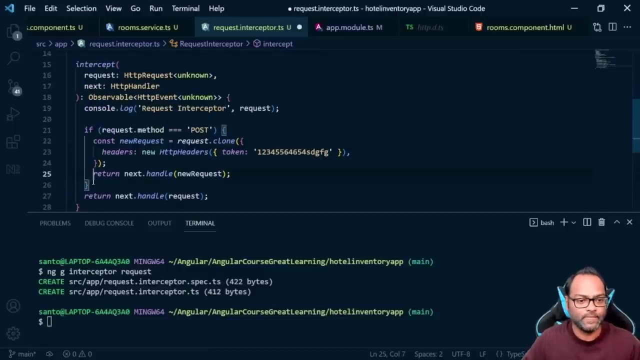 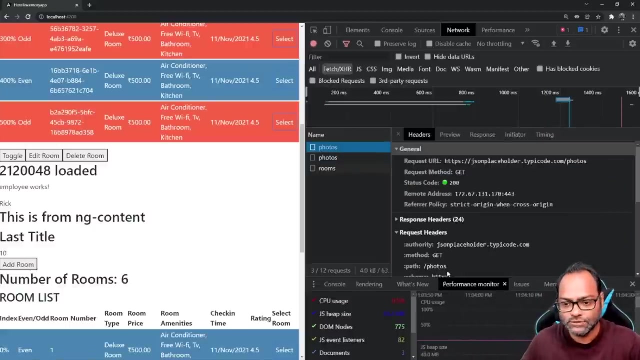 So I'm going to do this. I'm going to say, okay, if requestmethod is post, go ahead and add this token and make a request. otherwise make the original request. Let's format and right. So let's verify Now. our get request should not have this token. 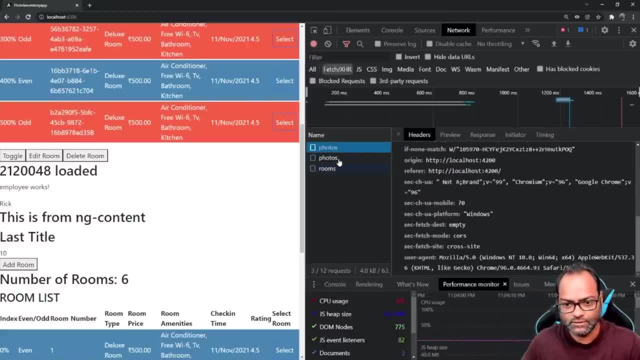 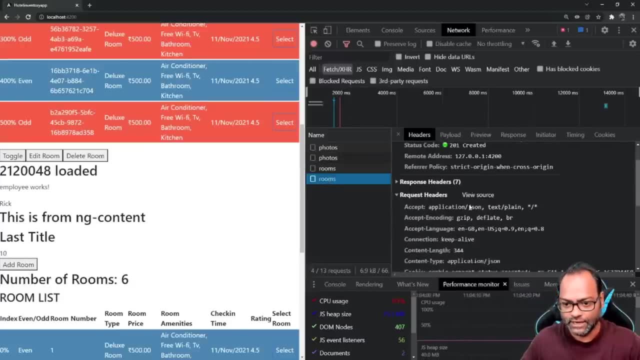 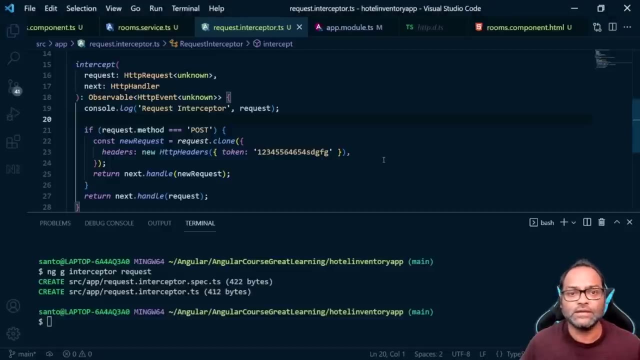 Let's go to photos and no, we don't have it. Rooms, We don't have it. Let's execute a post request by adding rooms, and now we have it. So these are the things which you can achieve using HTTP Interceptor. 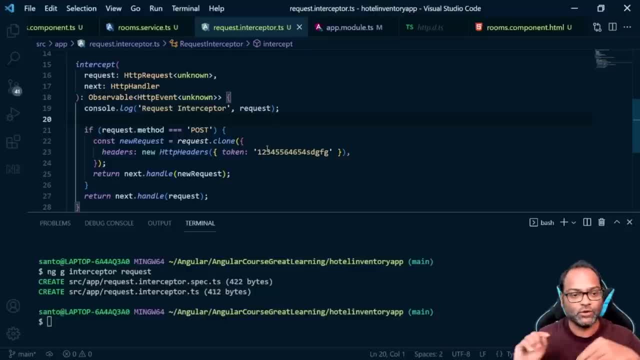 Right now we are only handling the request. Remember this. You can see I'm not handling the response. I'll show you one use case: while working with, probably, routing and forms, how you can also handle the response. So yeah, that's it from the HTTP Interceptor now. 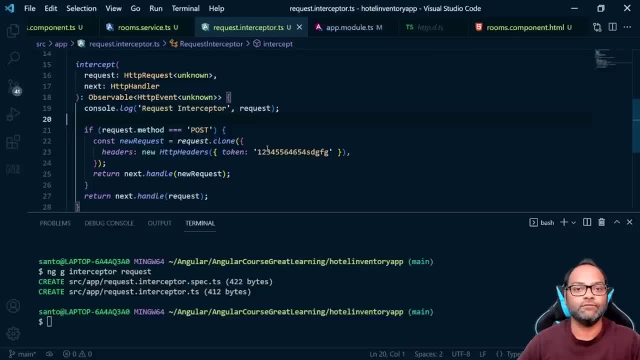 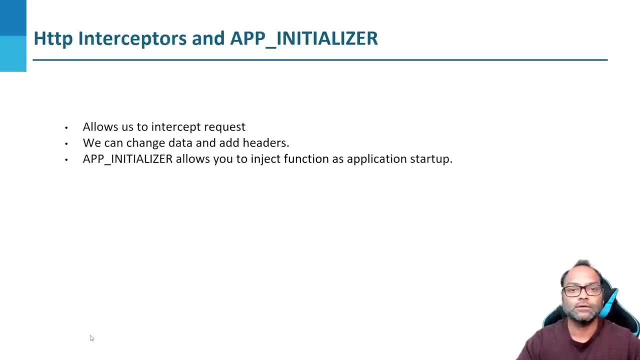 Next thing which we are going to talk about is: we will see App Initializer, So let's do that next. Next, we are going to do last topic from HTTP Interceptor- sorry, from HTTP- And we are going to discuss about App Initializers. 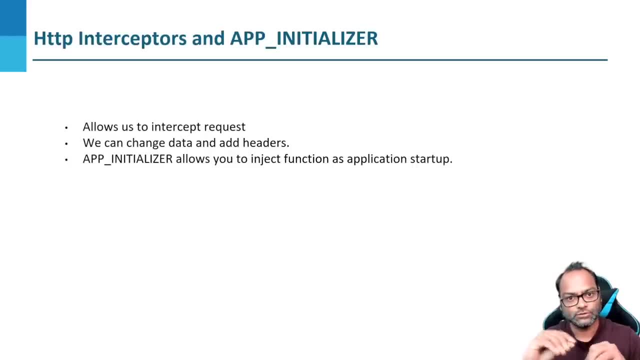 Now what and where you are going to use it. So this is a little bit advanced topic, as I'm trying to cover everything which you can. sorry, I'm trying to. I'm trying to cover everything which you can utilize in your production application. 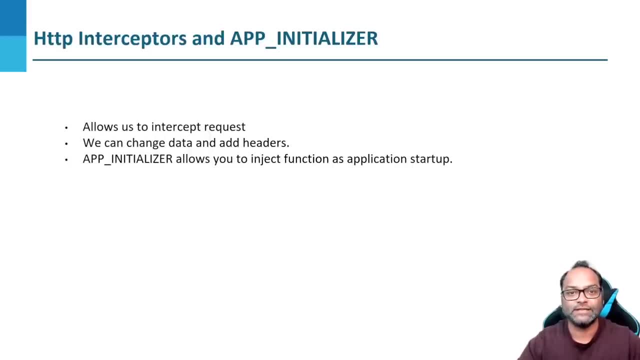 So you should not get any sudden things. okay, this is something which I'm not aware of, So this App Initializer is something which is really useful. It's kind of again a service which will help you to load the data before your app gets. 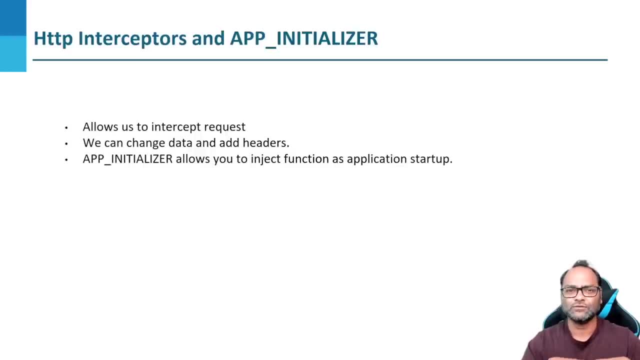 initialized. And now you might be wondering what is the use case when I need the data before app is initialized? You have some configuration. You need to load that configuration before your app is initialized, and then you need to save that data into your service and then use it. 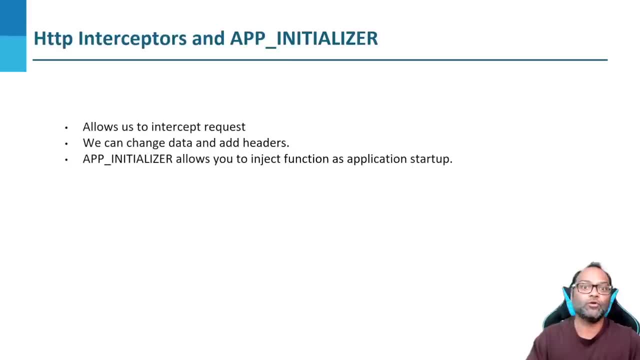 How you are going to do it. I'm talking about before your app is initialized, I mean before you get your first page. This is where App Initializer can help you. App Initializer can plug in your service and it will call that particular service before. 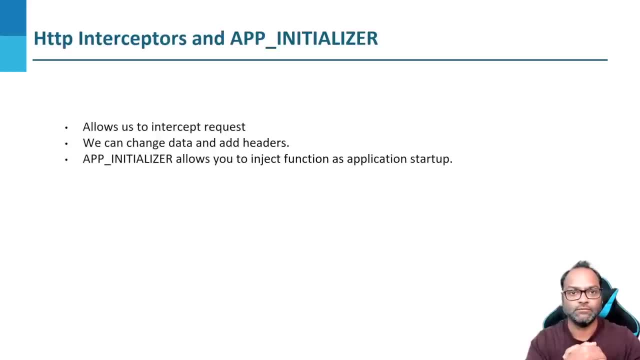 your app is initialized And you can do anything Where, whatever you want into that service. you can make an HTTP call, get the data from your any API, or you can just load a config file from your local disk, right? I mean, for example, if you have saved some file in your assets and you want to based 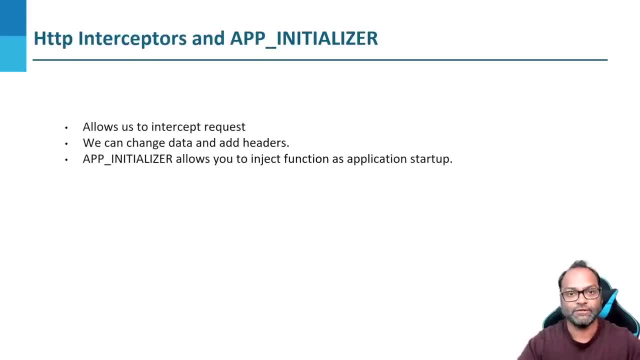 on your configuration. you want to load that asset file or config file. That's possible. So let's take an example where we will be using a config file and we will load that config file and we will make that data available before our app is initialized. 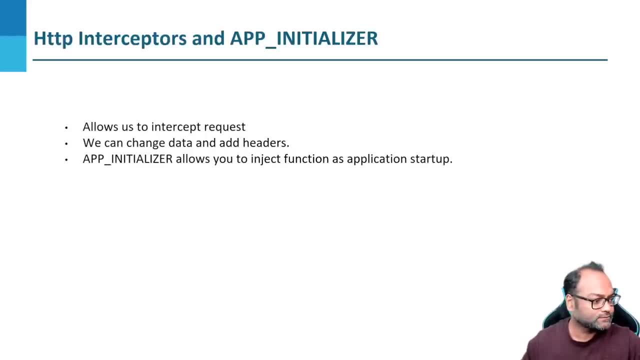 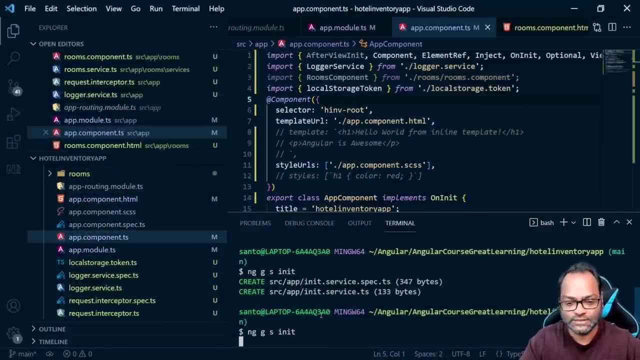 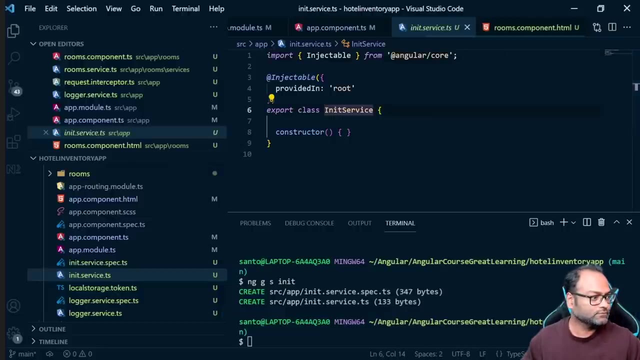 Okay, To do that first. what I'm going to do is I'm going to create a service, So I'm going to say nggs and I'm going to call it as an init service initialize, And I'll add some code here and we'll talk about it. 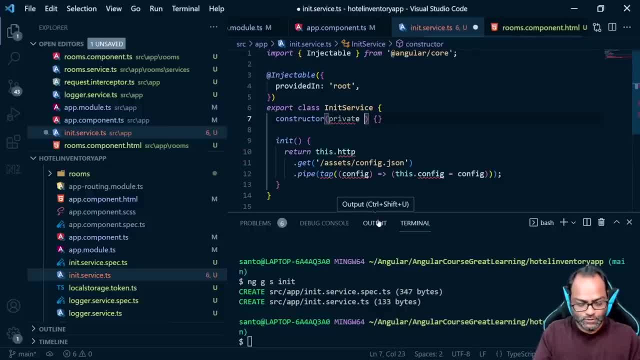 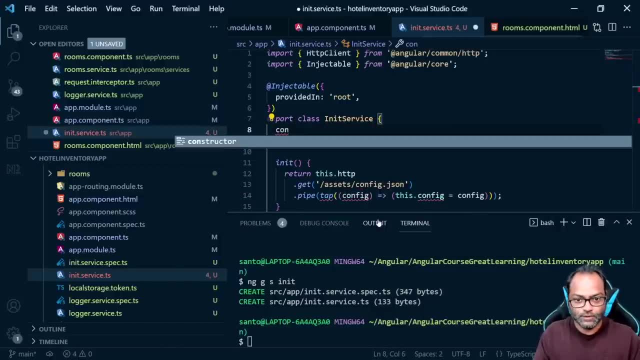 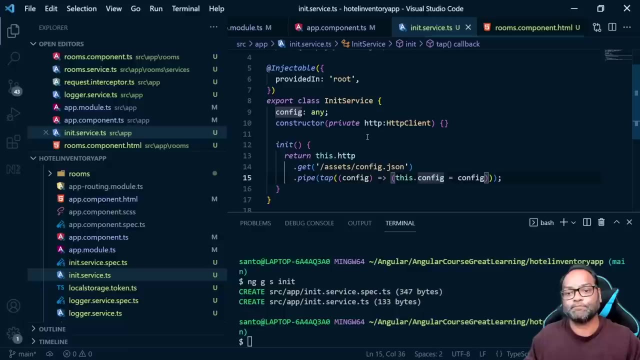 I'm going to make an HTTP call And we'll create a property which is type of any, and let's add this type of it. So what we are going to do is we are going to load this configjson file, which we don't. 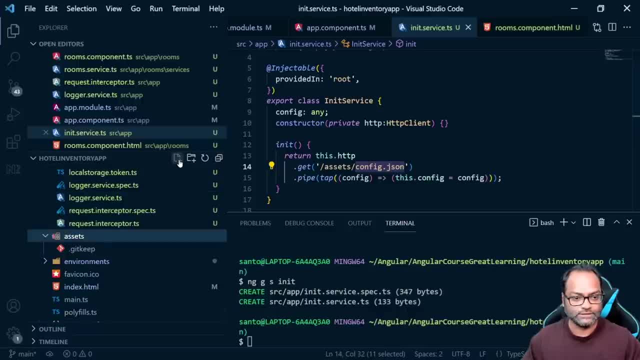 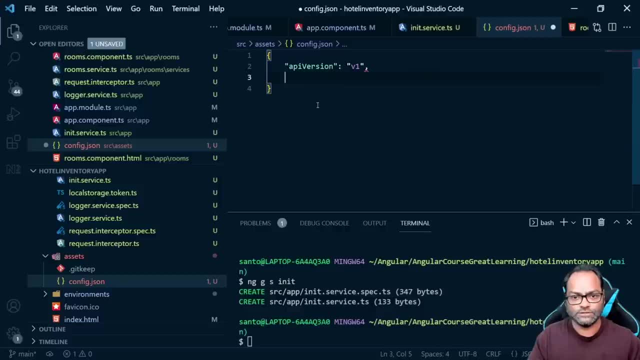 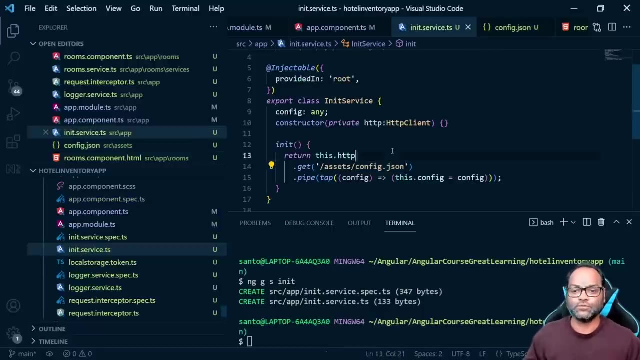 have right now. Let's create in assets configjson and let's add some properties, So let's API version and some some normal properties, right? So let's say it has two, these two properties as well. Now this service needs to be called before my app is initialized. 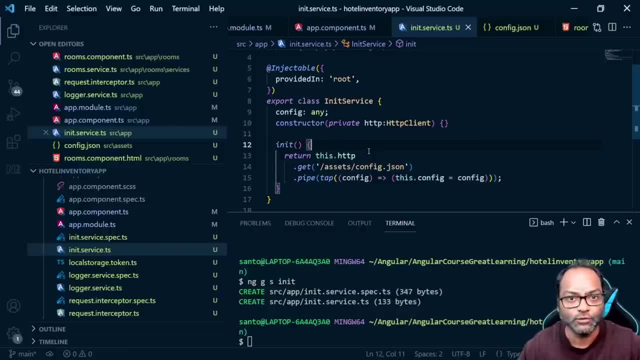 So I can make the HTTP call, get the data and do whatever I want to. I mean, I can just go ahead and use this service anywhere and the data will be available. Now let's see how to use it. So that's a little bit change in the syntax. 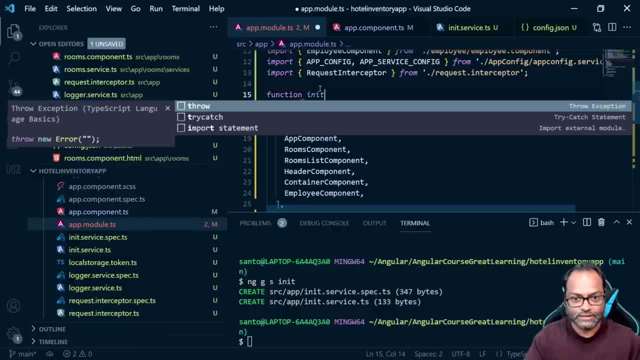 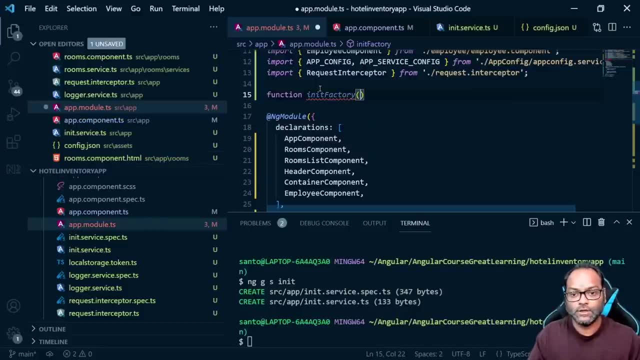 So we are going to create a function, We'll call it as the init factory And we'll pass our service here. So we'll say, okay, this is a init service, which is type of init service which we have. And then we are going to say: return a function. 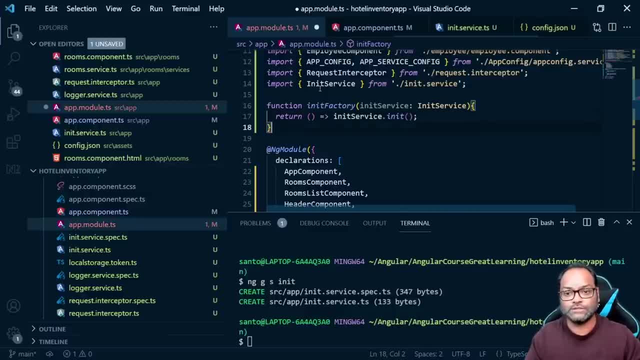 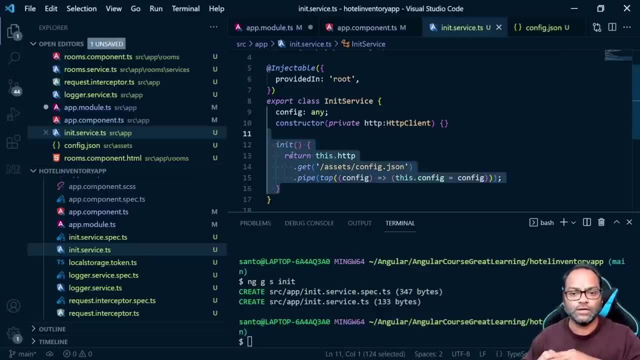 This is a really important part. So we are going to return a function which says init service dot init method, which is the method which we have here. So this method will get: make an API call or HTTP call. load the JSON file. 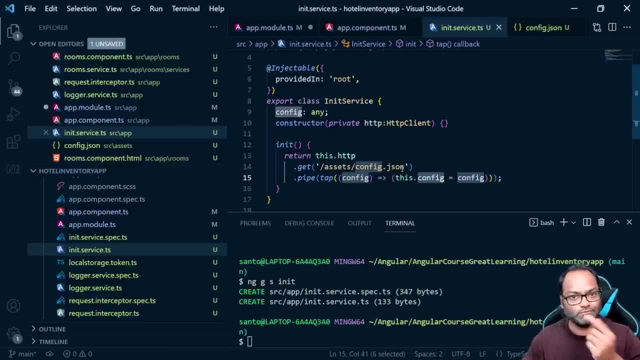 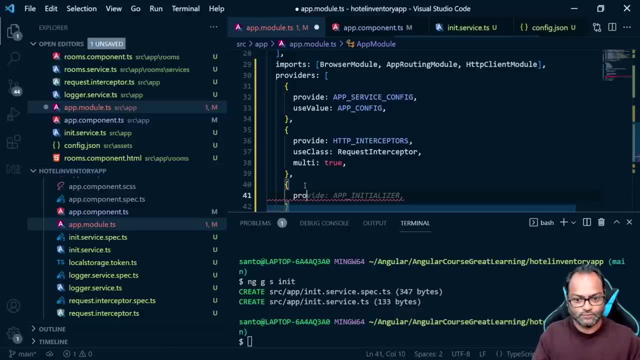 And add: save this into this particular property. Now, once this is done, we have to register it. To register, we are going to say provide app initializer, because that's a service where we want to actually plug in this particular method. 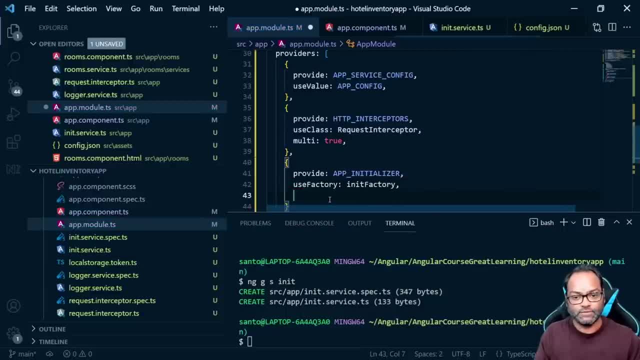 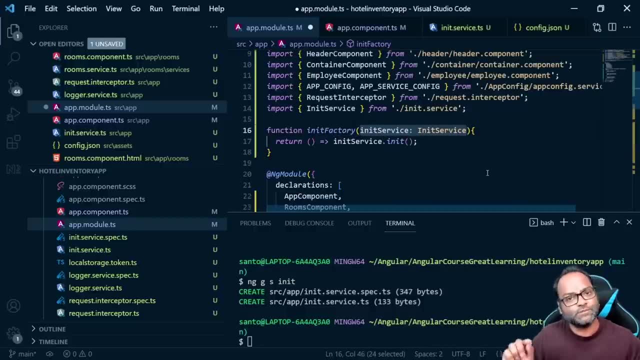 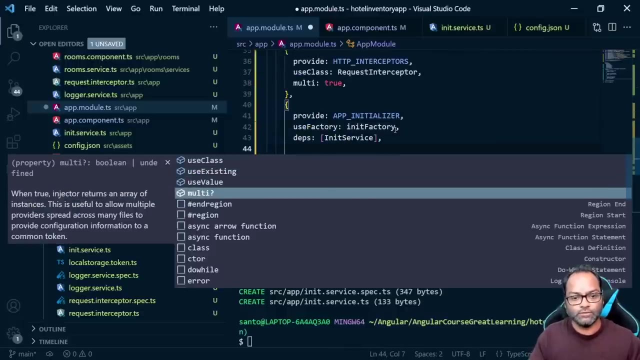 Then we can say: use factory, as we have factory available. Then we have to provide dependency. Dependency will be the number of the services which you provide here. It's possible that you can call multiple. That's possible- And you have to say multi-true, because app initializer is again an object where we are. 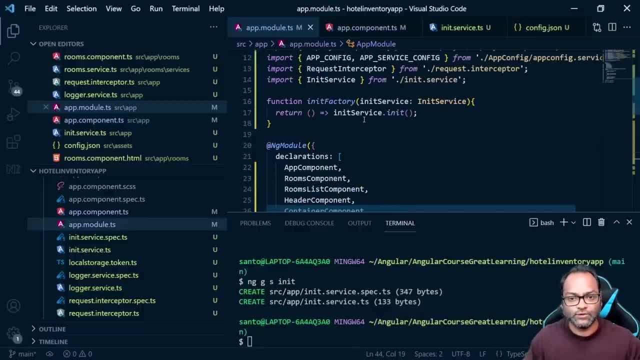 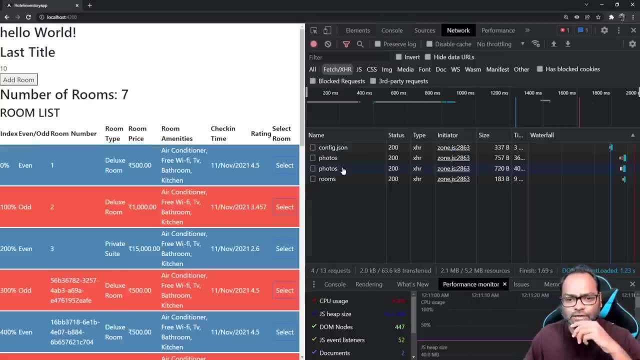 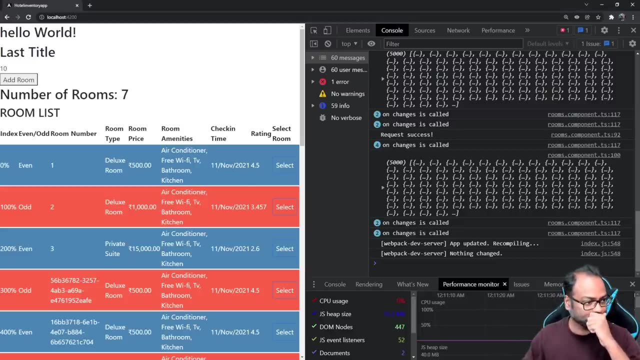 going to add our service. Now this is done, Let's go ahead and verify if this works or not And how we can verify. just going to the network tab and configjson is loaded. Yes, that's loaded. Let's try to read the property. 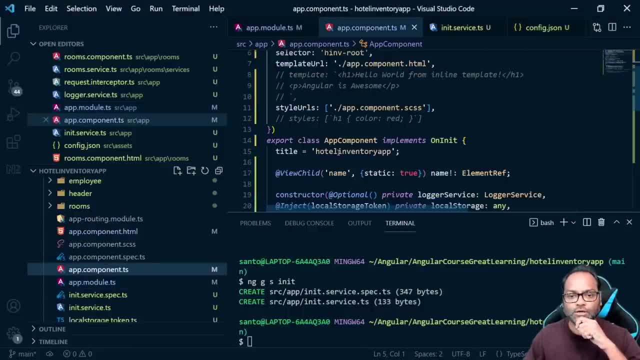 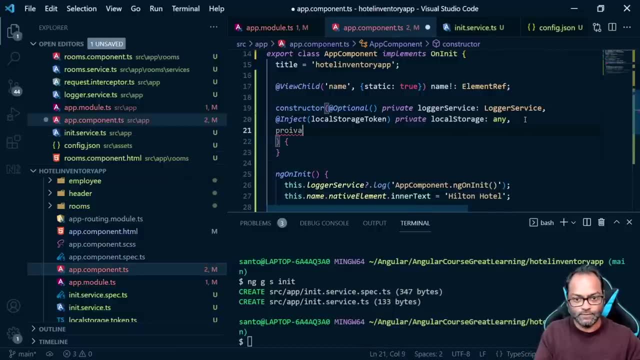 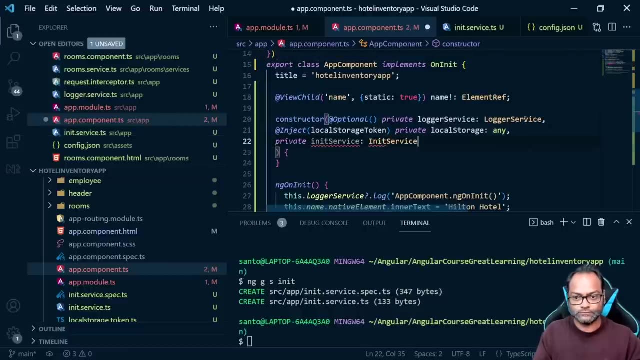 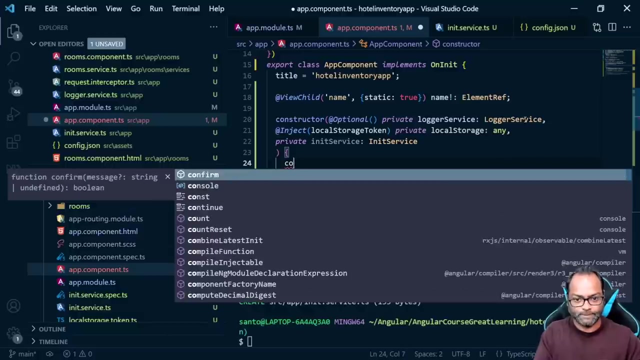 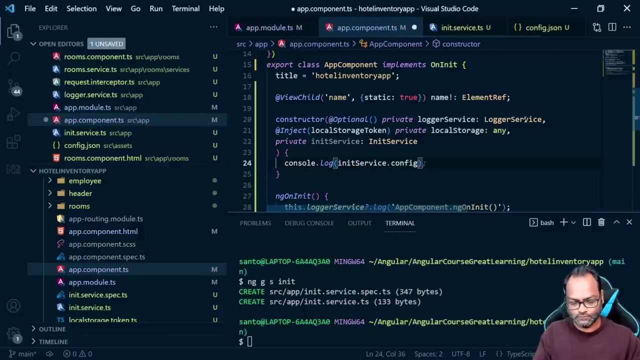 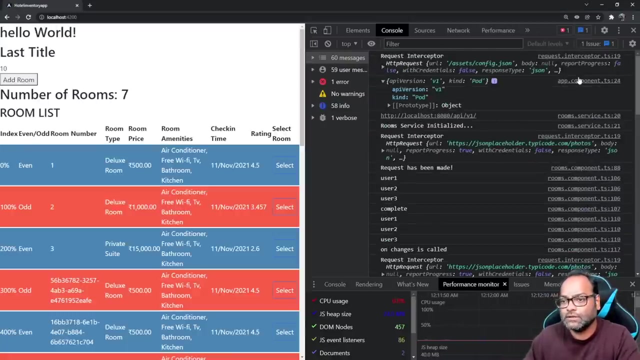 Now to see if this property is available. If this property is available or not, we can inject the service in here. So let's say this is private And we'll just do consolelog here, serviceconfig, And let's verify: And we have this data available- appcomponentts24.. 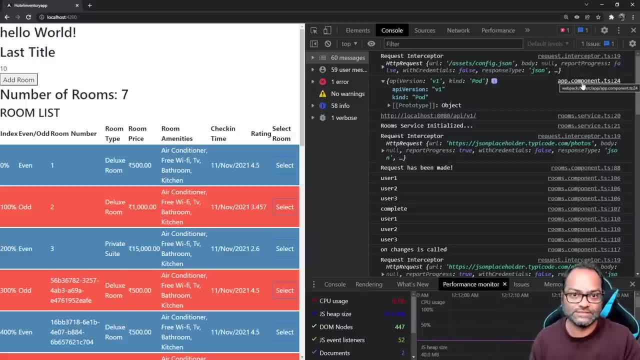 And this is available, And this is loaded even before your app is initialized. So, yep, this is how you can do it. Common use cases: maybe, let's say, you have a configjson file where you have environment APIs based on your environment. 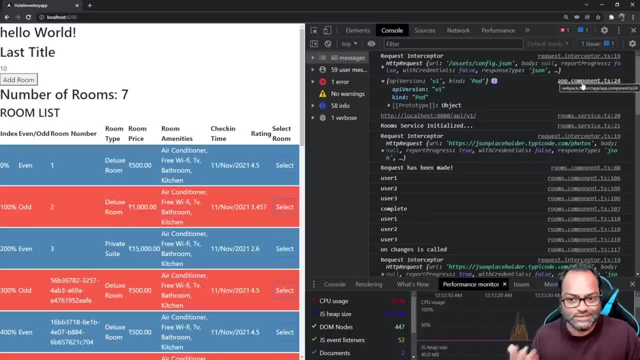 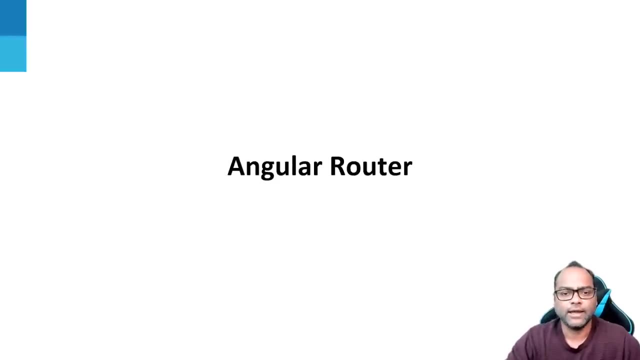 And you want to load that and then make API calls? Yes, that's how you can do it. So this is the last topic from HTTP, And now we will continue with Trouter. So far we have learned about the basics of Angular. 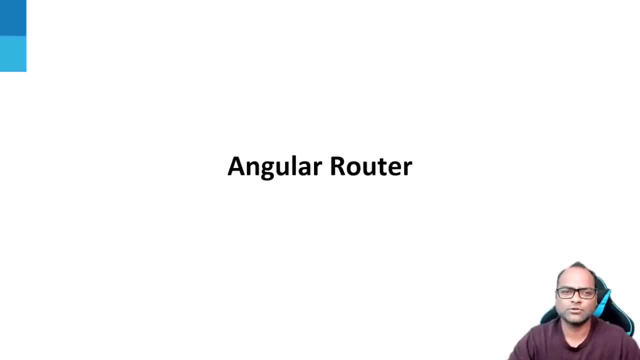 And one thing you may notice is we don't have so much of UI right now available. We said we are going to use. we are going to create a project based on Hotel Inventory, But we just have like a table and we saw some functionality where we can add details. 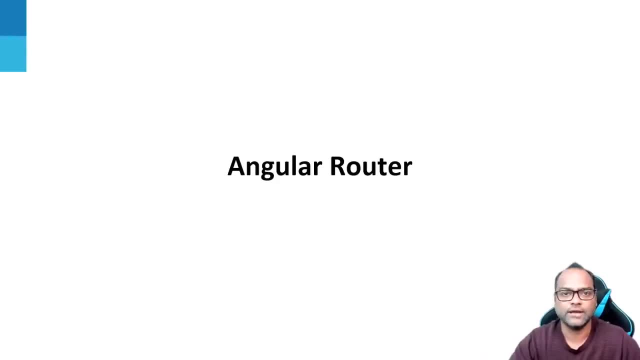 And that's it. We can edit, but we don't have forms, We don't have URLs where we can click and move to different views. So this is what we are going to start right now. We are going to start with Angular Router. 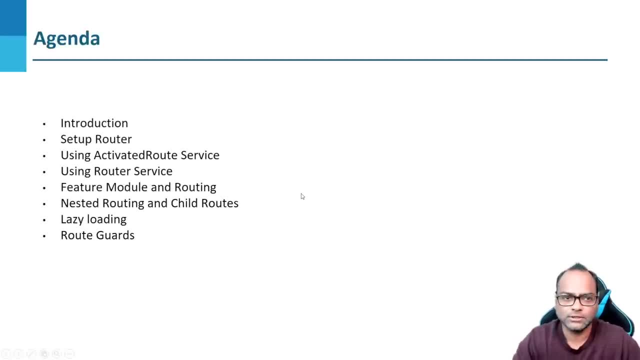 So in this video we will talk about the introduction, of course, and then we'll see. we'll see how to set up router. We will also see some services which is provided by router itself. So we have activated route router service. 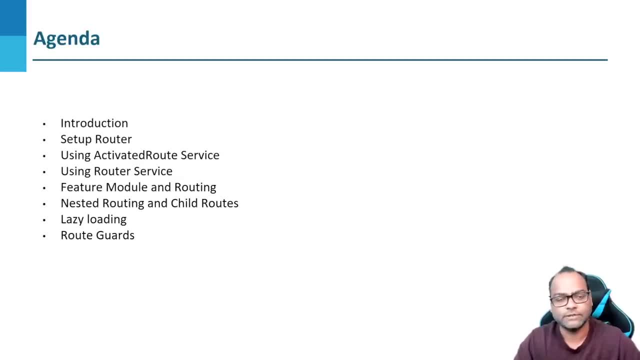 We'll talk about feature module And we'll we'll see- Okay, We'll see- how we can do feature module routing as well. We'll talk about nested route, child routes, lazy loading, route guards. We'll also see. if you remember, in last session we, in last video, we didn't cover how you 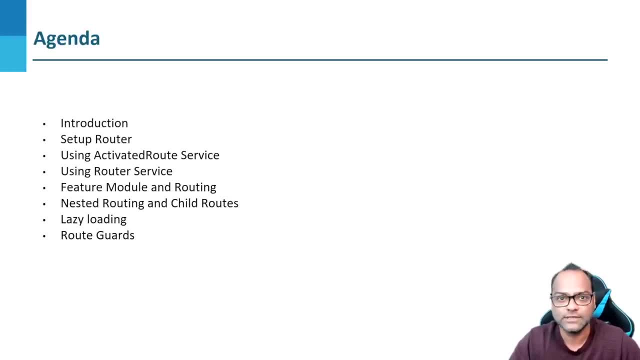 can communicate between, between multiple components using services. So that's what will be covered in this, this part as well. we'll see how we can do that, And we'll also see Angular material. So let's go ahead and get started. 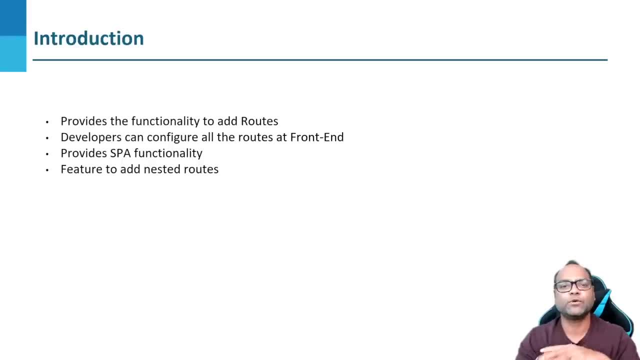 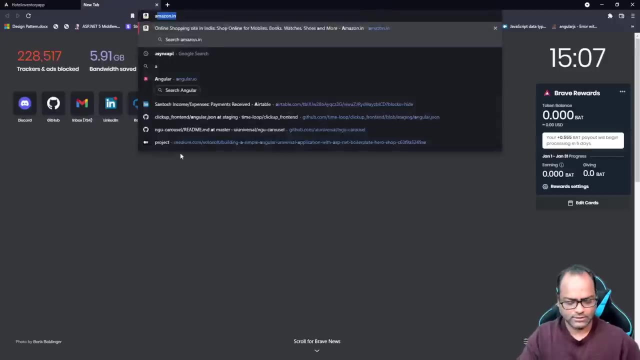 So let's see what Angular Router is. So it's provide it provides the functionality to add routes. I mean, what is the routes right? So first we have to actually go ahead and understand what the route is. So let me show you a page and I'll go to angulari. 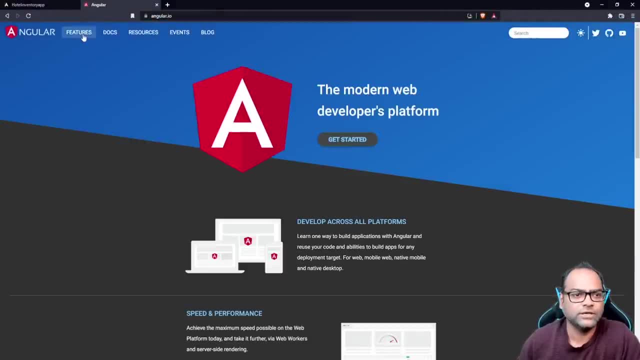 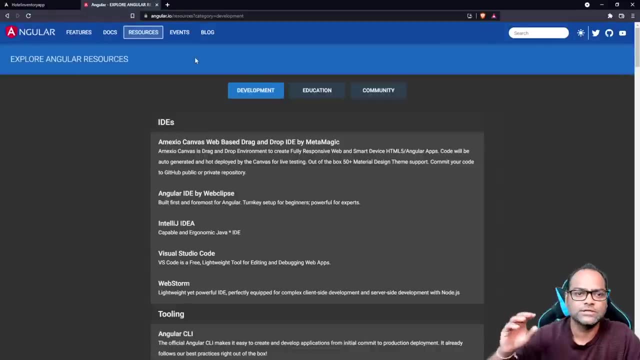 So the documentation right. So here you can click on features, You can click on routes. These are different, Sorry. You can click on features. You can click on docs, You can click on resources. So these are different routes which are available on this page. 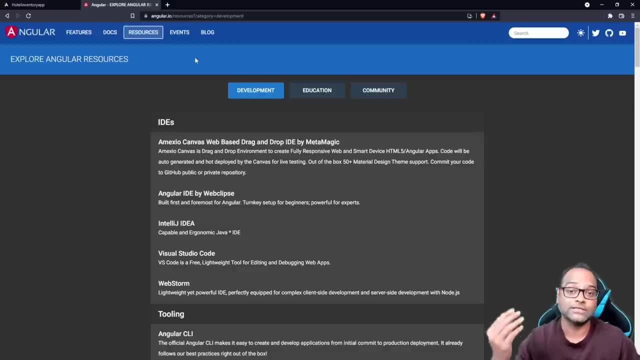 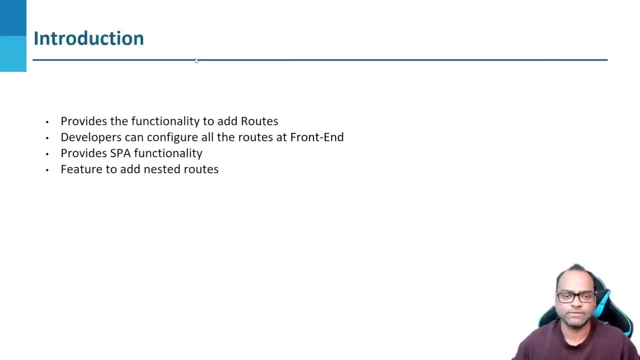 So, using Angular Router, we will be able to configure all this on the front end itself, So we don't have to do this on backend. It provides this SPA functionality, single page application. So, if you see, we are still on the same page, right? 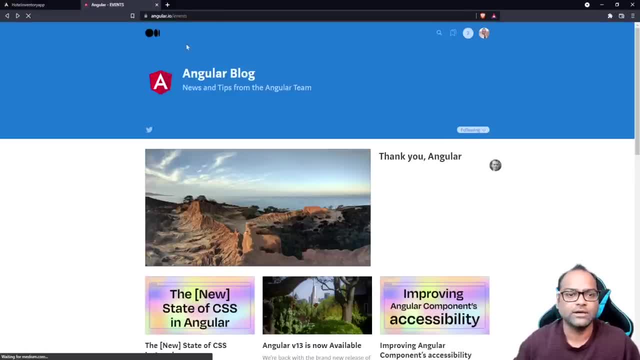 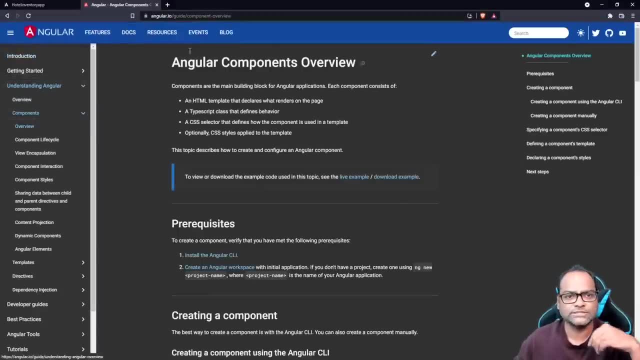 If you click on blog it redirects to another page, So this is different. but this is single page application. So where you can click on any- let's say we can click on docs- You can click on any of the URLs or you can see URL is getting changed, but there is. 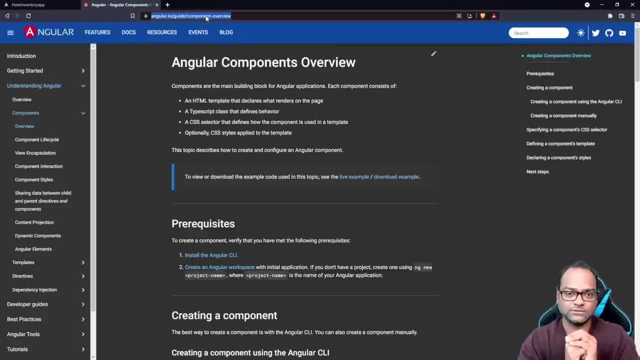 no request to the server. So everything is happening on your front end, which means it's a single page application where everything is known to your application in advance, So it doesn't need to take any data from the backend apart from the HTTP calls which we. 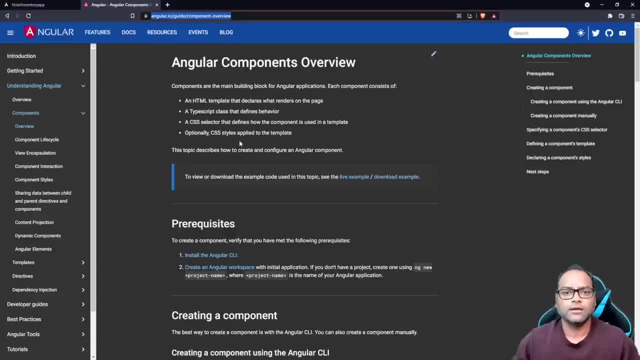 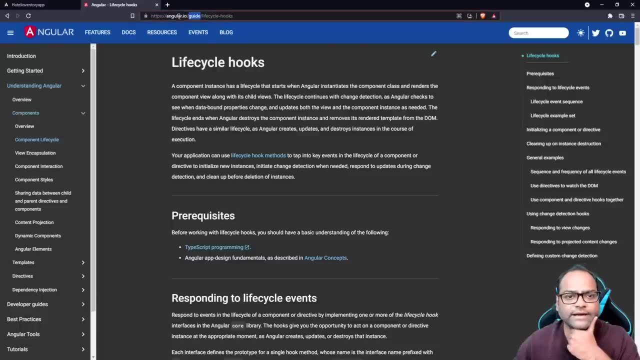 will be making Okay, Okay, Okay. So let's talk about the other nested routes. So what is the nested route? So you can see. if I click here you can see guide is the main route And then in guides we have different. I mean, this is not, this is not the child. 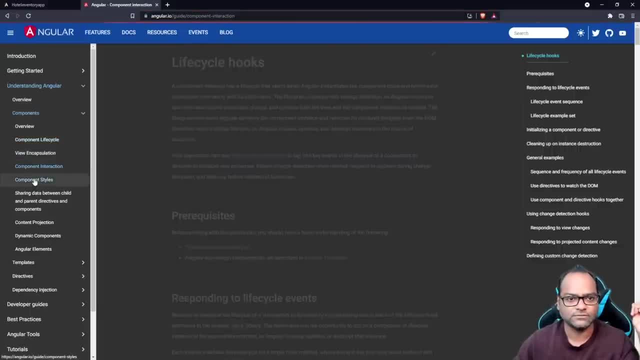 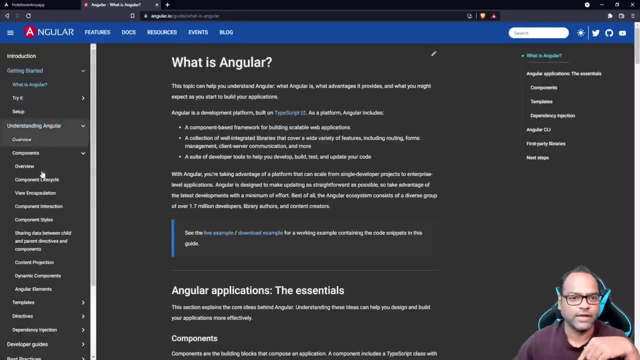 So you can see guide is the parent route and then you have different child routes available inside this. So if I go to get started, you will find okay, what is Angular developer guides. but yeah, I mean everything is getting loaded inside the same route. 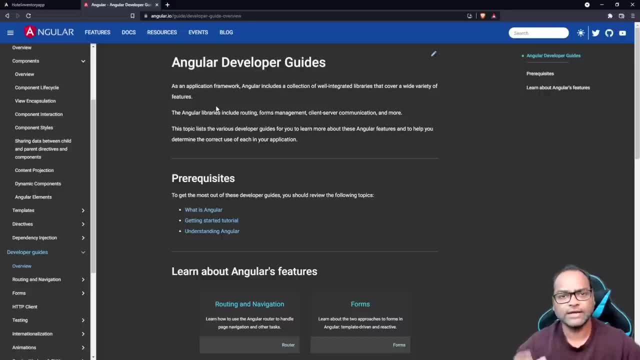 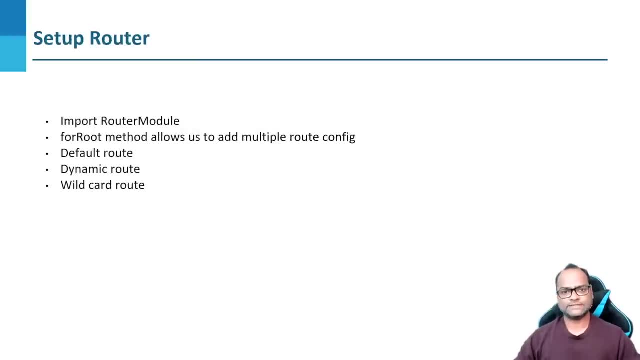 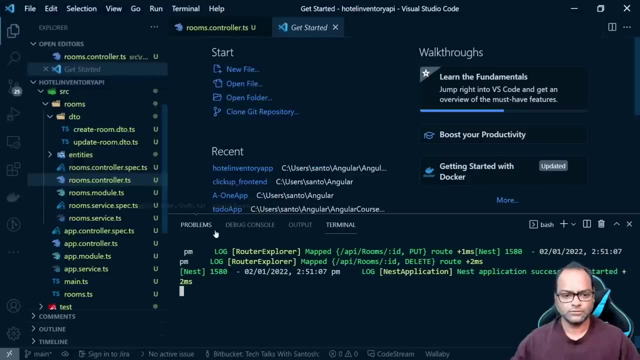 So you can see how we can also configure something like this, where we can replace some part of you. So that's, that will be covered as well. So let's go ahead and see how we can set up router. So let's go back to the code. 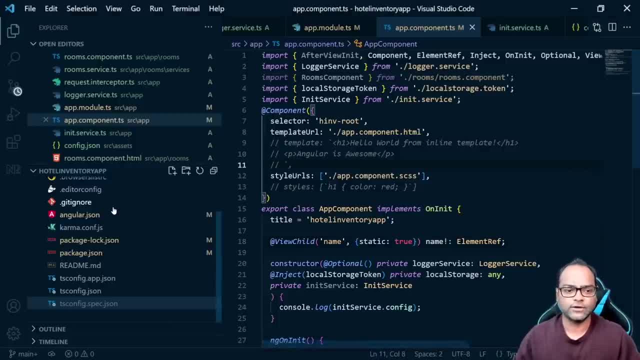 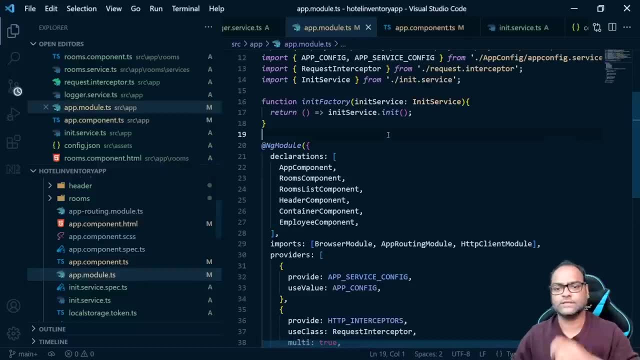 So this is our code and we don't have any router routing functionality as of now, and let's go ahead and add that. So we'll be adding it inside app module. Let's see what needs to be done. Let's go back to the slides. 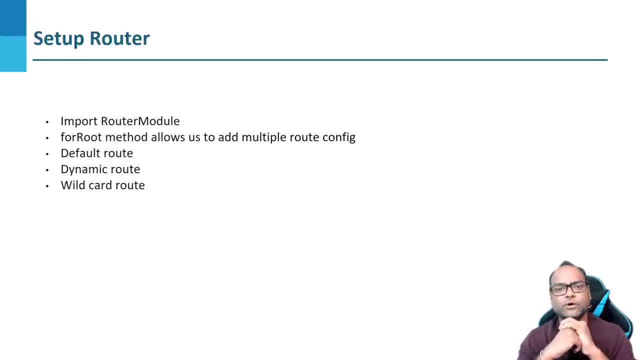 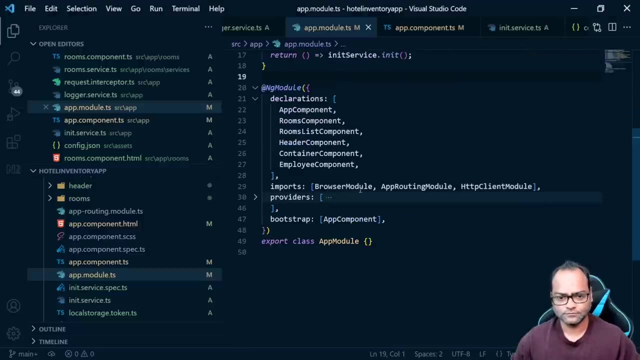 So what we have to do is we have to first go ahead and import router module. So router module is the module which will provide us all the functionality required for or required to use the routing functionality which Angular has. So let's add: 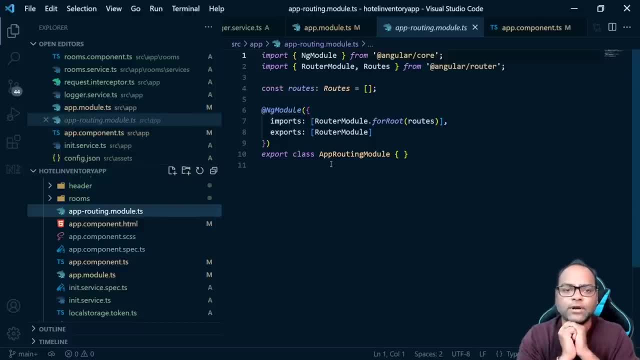 So I'll not do it here. So we already have something called app routing module. Remember, when we created this application, there was a question using ng new. So there was a question: do you want to configure routing module? And we said yes, 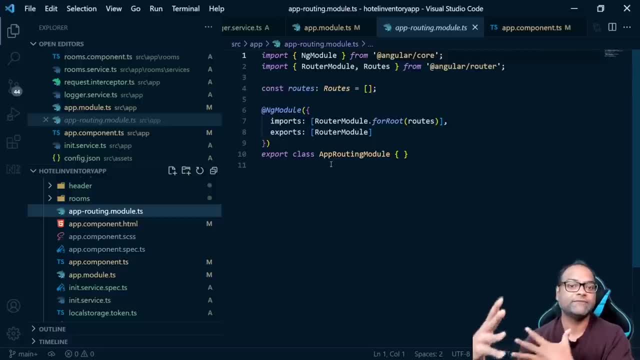 So that's the purpose, So we can keep our code in different modules. So here this app routing module is to configure any routes which we want to configure. So we already have this. So you can see we already have router module imported and then we have exported it. 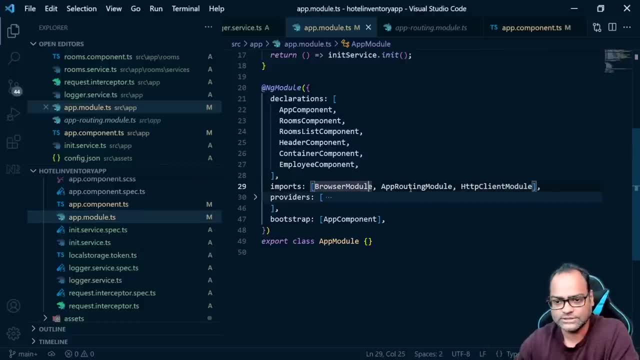 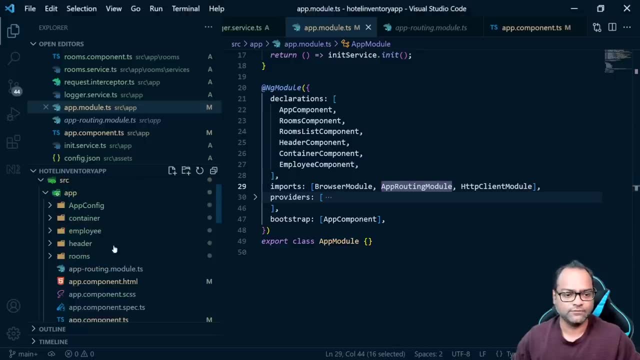 So my app Component, So the app module, knows about this. So you can see, app routing module is already added here, So this step is automated now. Then we have for route module, So let's see for route function. So here it is for route. 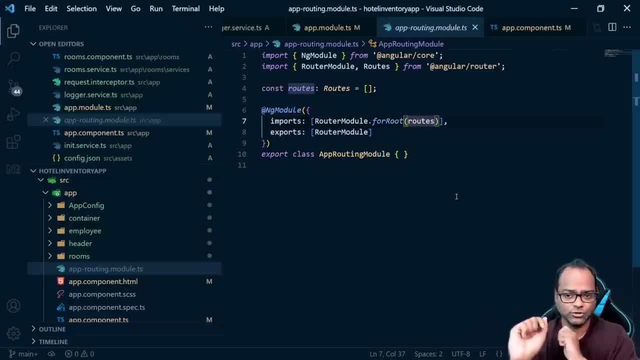 So you will be configuring for route only once. Remember this: you should not configure for route multiple times. It's single term service. So, in case you do, it will probably override the previous routes which we have added. So this is taken care. 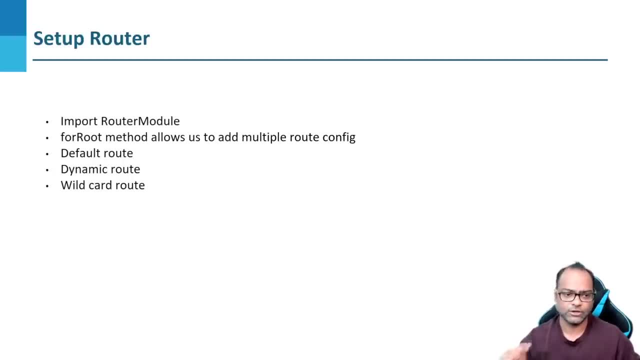 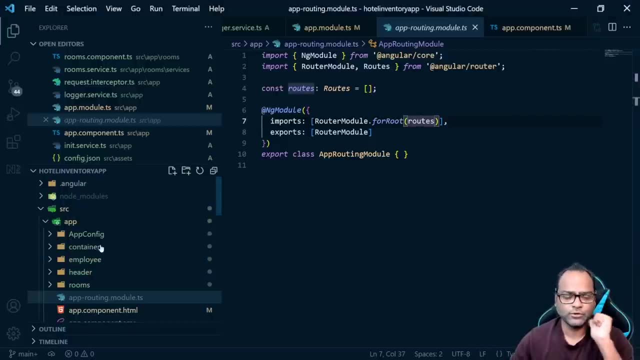 So for route is also available, And then we will talk about default route, dynamic route and wildcard route. So let's go ahead and see first how we can configure the routes. So what we are going to do is we are going to create multiple URLs, as we saw on angulario. 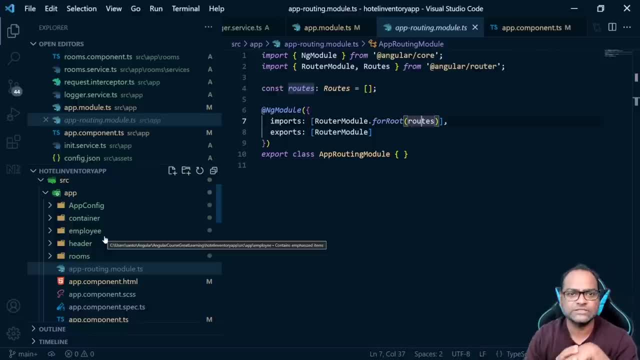 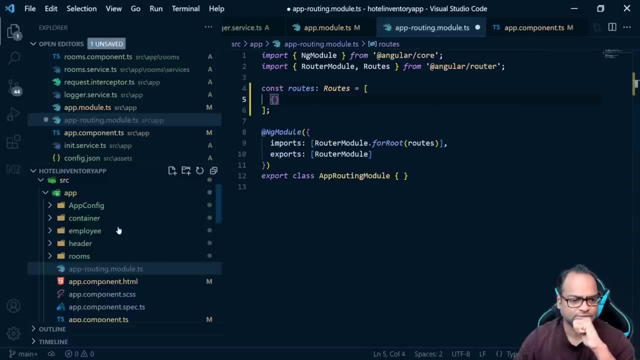 where you can click on guide, we can click on docs, we can click on features, and it moves to different UIs. So let's see how many components which we have right now. Sorry, So we have this, employee rooms and container. let's just say we have three, this three. 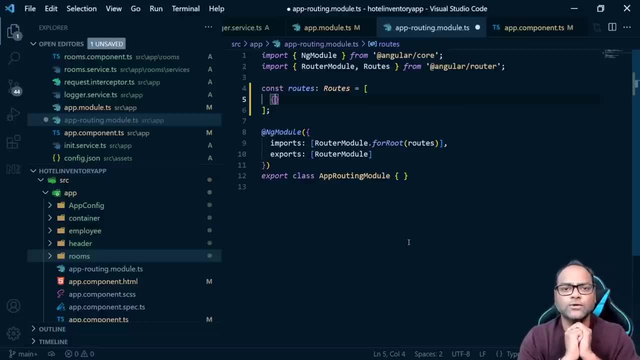 So let's see how we can configure a route. So to configure a route you have to pass two things. So first is you have to provide a path. So we will say, okay, this is path and you can give any friendly URL name you want to. 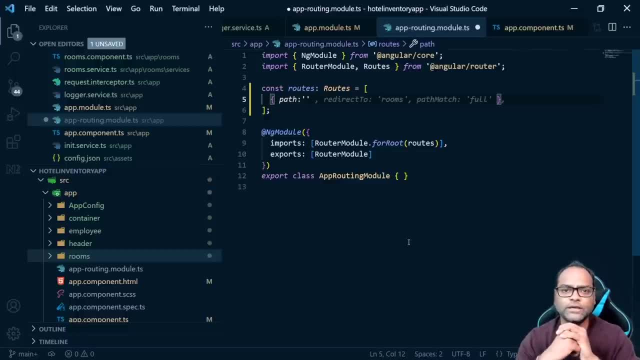 For example, if I want employees component to be rendered, When I click on render Okay, I click on a URL called slash employee. localhost 3000, sorry, localhost 4, 2, 0, 0: slash employee. 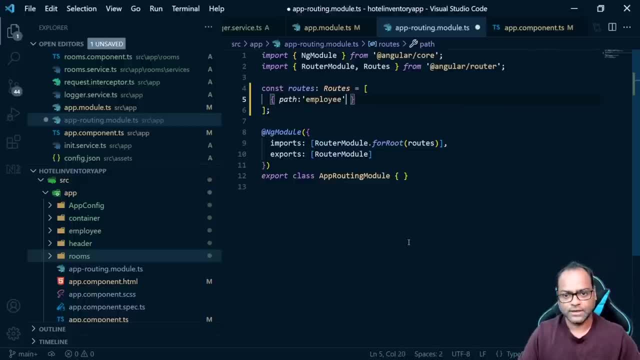 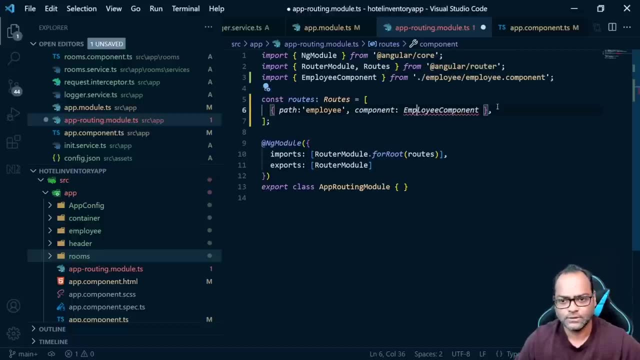 I can do something like this, So I can say employee And when I click this, this, go ahead and give me employee component. So first is configured. we will similarly do it for this. So let's say path and we'll say rooms. 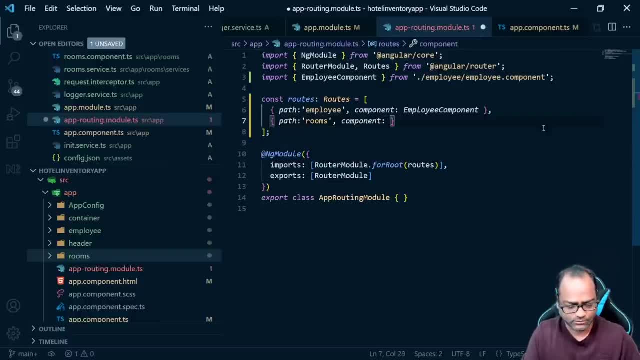 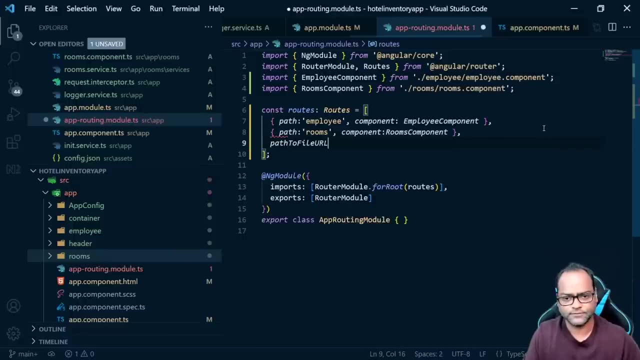 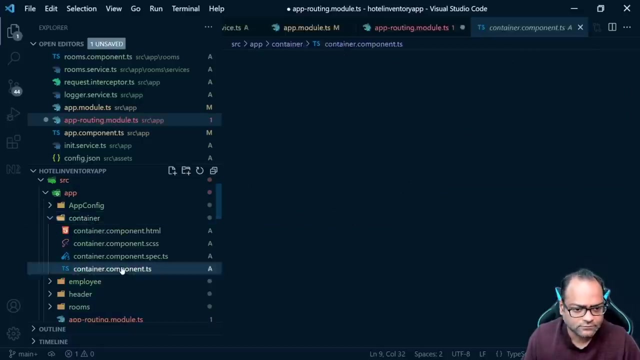 And when I do this, I want this rooms component to be rendered. And the last one is: I want this to be- let's call it as container as of now, And when I do this, I want component, but one second, Okay. 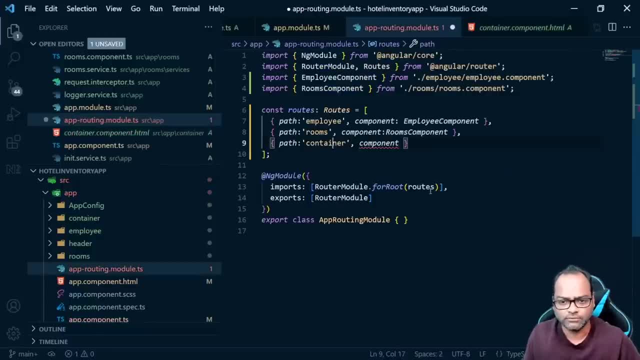 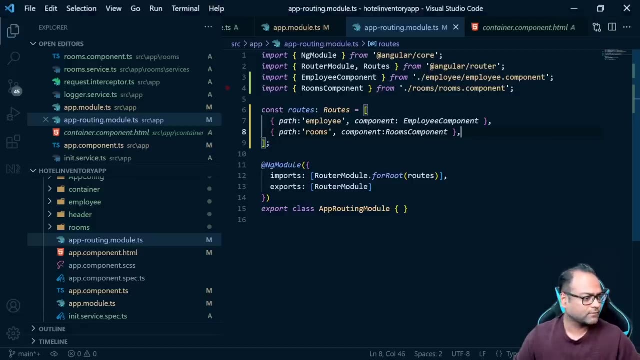 Container component will not render anything by default, So I'll just remove it. I'll keep this. So we have two routes available right now. So employee and rooms, And let's try to see if our application works. And let's say rooms. 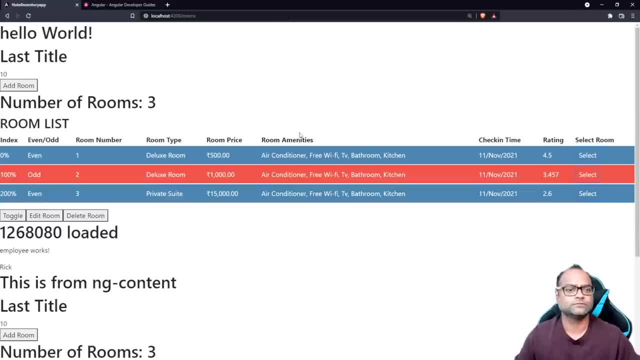 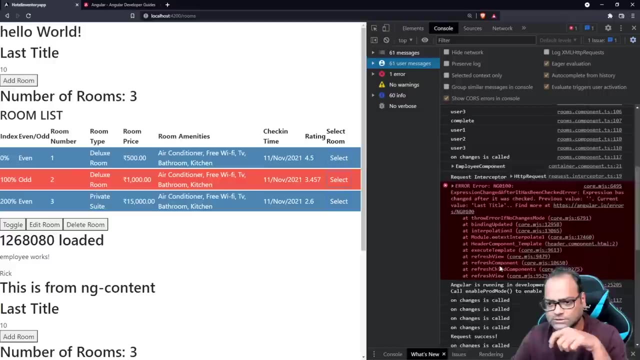 I entered the incorrect URL and it doesn't Right. It goes back to whatever view we had. So let's see So there should be an error, Let's see So. okay, Right now. Okay, That error is because, okay, this route is okay. 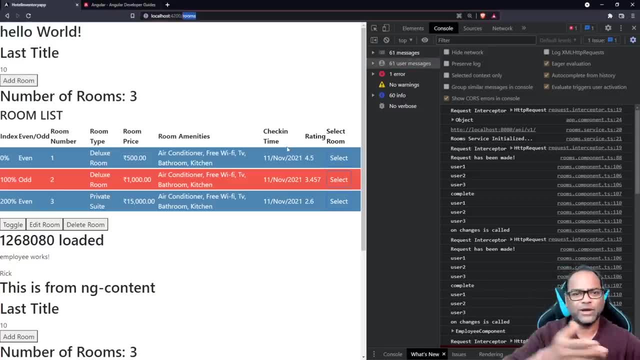 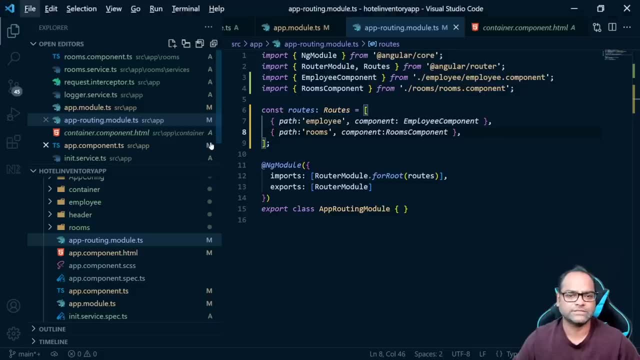 So when we are clicking on slash room so you can see, okay, there in UI you can see the URL, but nothing happens, Right? I mean, so it should only display the content related to rooms. Or when I say slash employee, it should only display the content related to employee. 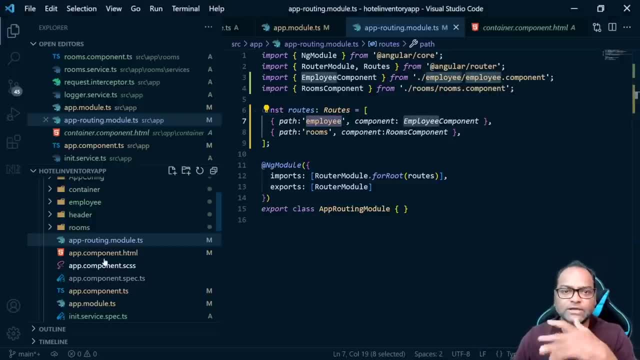 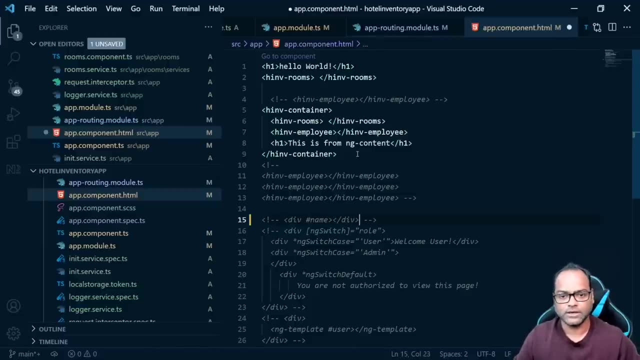 Because we are missing one important thing. When we configure routing, we have to place- So I'll just remove this, I mean, I'll just comment all this out here- And container- Let's remove this, Let's remove this And let's remove this as well. 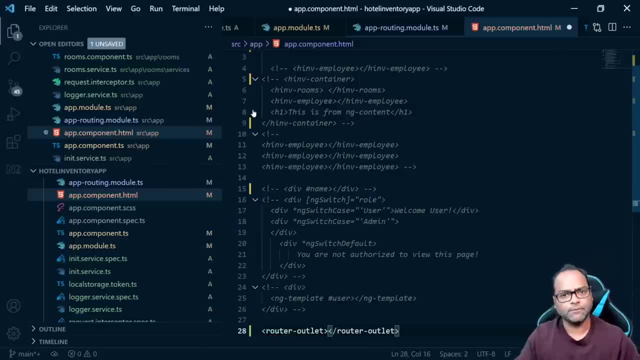 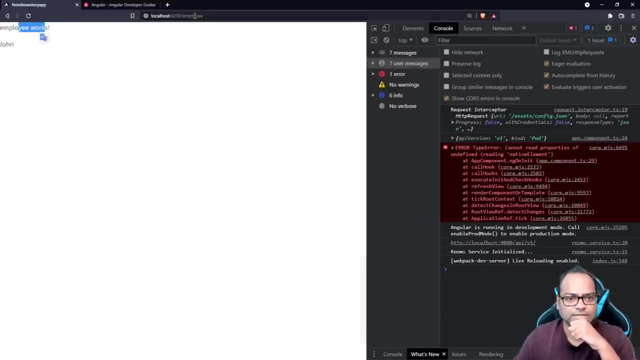 So here we have to place something known as router outlet. I'll come back and we'll talk about this, What this router outlet does. And let's see. So we have so slash employee and it says employee works. And then there is John, because this is what it is available on employee component. 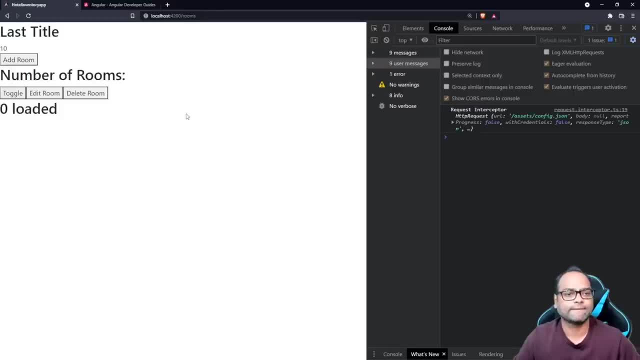 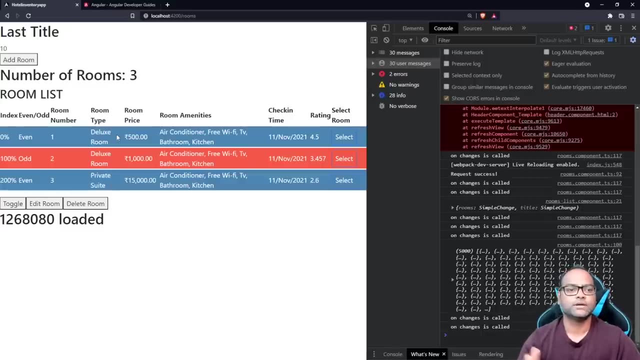 That's it. Let's try with rooms And you should be able to see all the details related to rooms. It works. I mean sorry, So it was. I mean so we have rooms related data When we click on rooms. 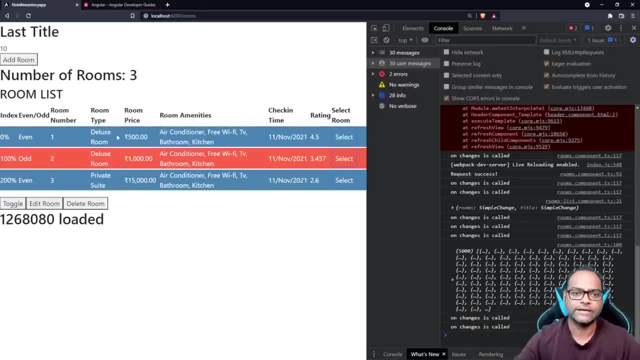 We have Employee related view or we can say employee related data when we click on employee. So we have configured a route, but do you think this is usable? The answer is no, of course. Right, I mean, generally we don't do that. 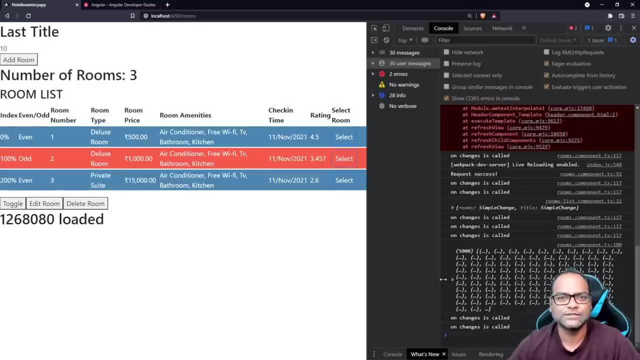 We don't ask users to go ahead and click on this URL So you will go to rooms, or click on this URL So you will go to employees. We don't do that. We generally have a nice navigation available or, whenever you do, localhost 4, 2,, 2, 0,. let's. 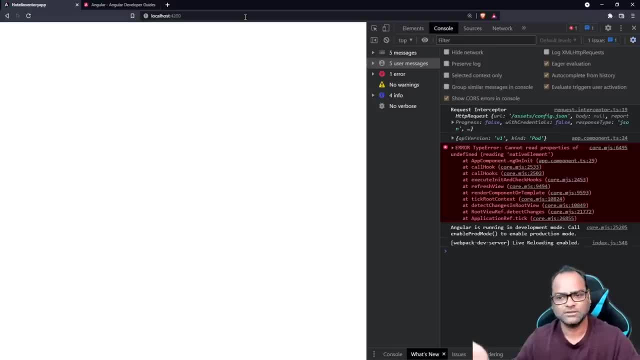 see this. So 4, 2,, 2, 0, and nothing happens. There's nothing available on my route. So, generally, what we do is for this, we set up a default URL. So what we'll do is: let's set up a default URL. 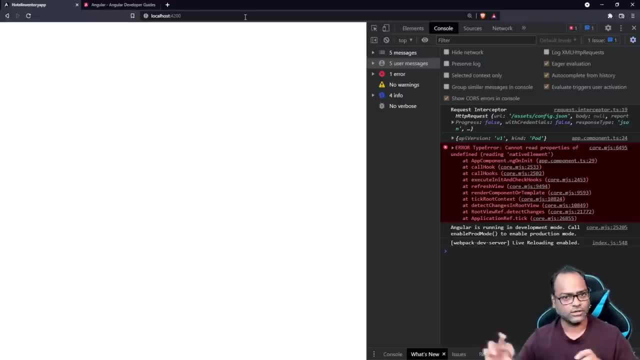 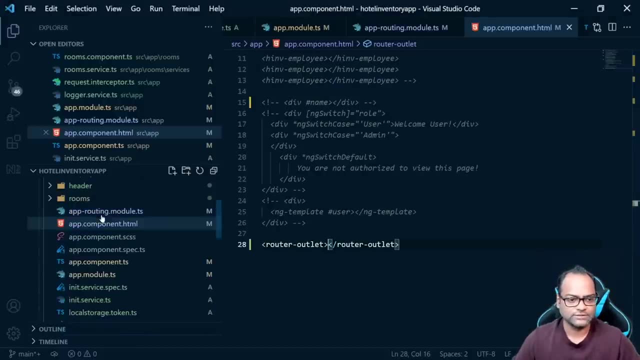 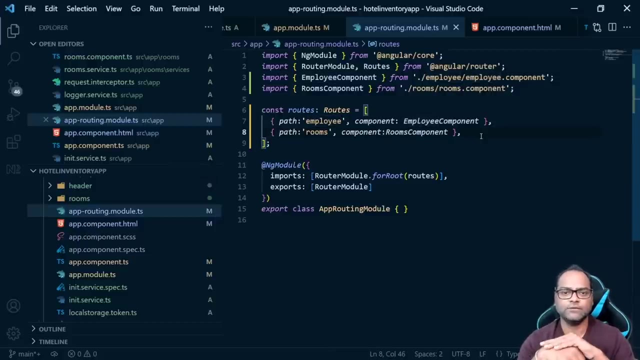 Then we will see how we can work on the anchor links or the URLs, and then we will add an angular material. So let's go back to the code and let's do first thing. first we will add the default URL. So what I want is: or as a user, as a developer, what I want is: I mean, uh, whenever a user 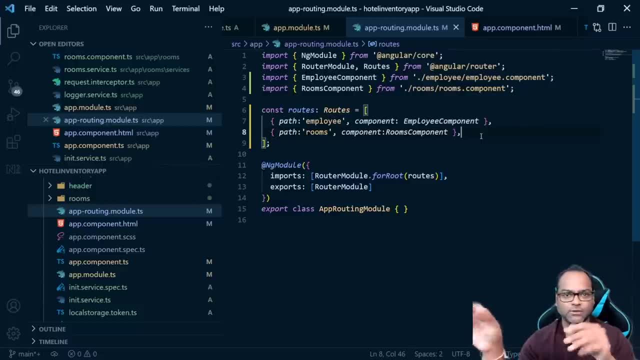 comes onto my page. let's say he enters wwwabccom or, right now, localhost, 4,, 2, 0, the user should be redirected to rooms. So how we can do that? So we can say path and redirect to slash rooms and path matchful. 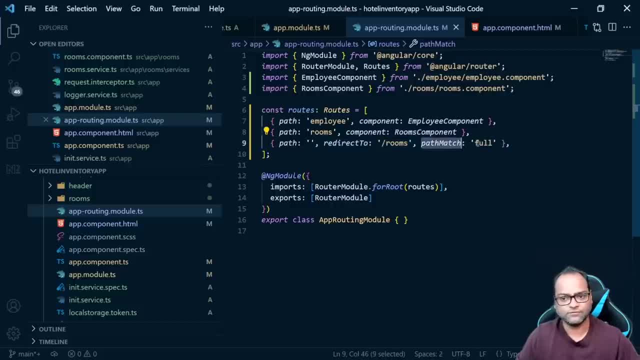 So it will match the entire path. That's. that's what this path matchful means. You can also provide regex expression in case you need to. Users of the application don't need that, So don't overcomplicate things. So here we are saying: okay, whenever I come, whenever a user comes on my webpage and there. 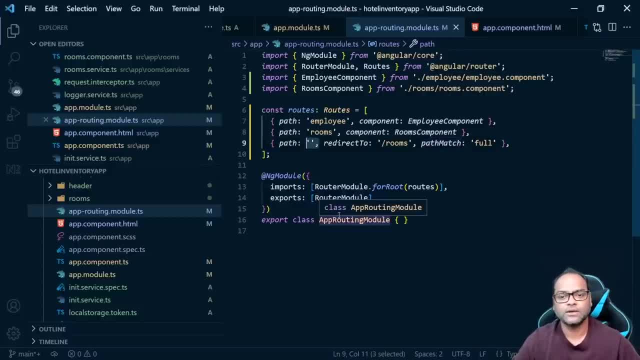 is nothing after that. slash 4, 2, 0, 0.. So the path is empty. redirect to the rooms, which is already configured, and make sure that you are matching full path. So let's see, And now we are redirected to rooms. 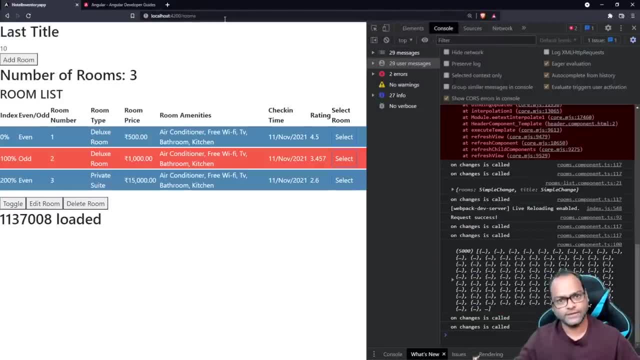 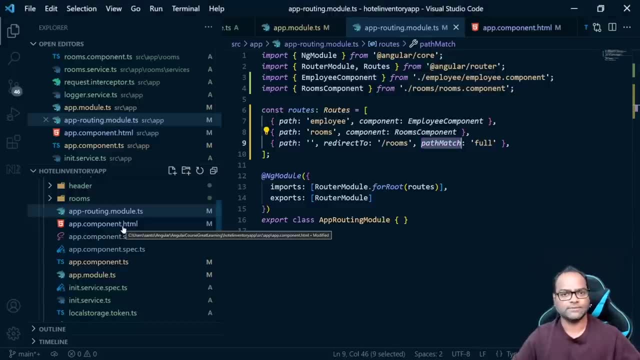 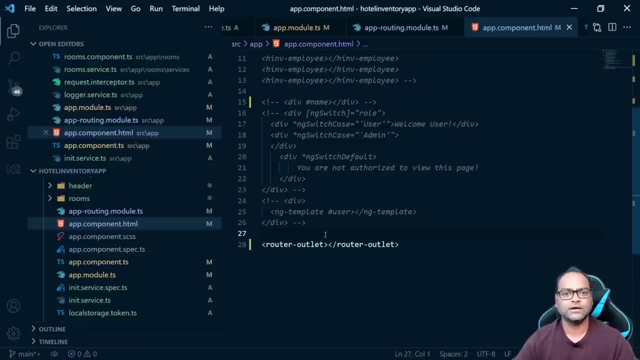 Let's go ahead and verify it again: 4, 2, 0, 0. And we are redirected to rooms. So this is how the default URL works. Now let's see how we can actually add some navigation. So first what we will do is we will add some anchor links, and then we'll see how we can. 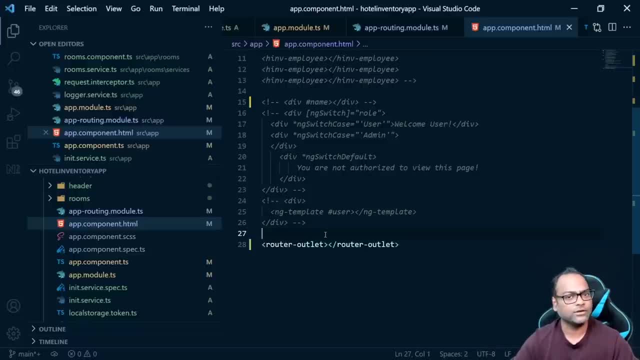 ease this process by using Angular material or any other URL of your choice, So I'll add anchor Now. you may have used href. Don't use href here, So let me show you what happens in case we use href. Uh, so 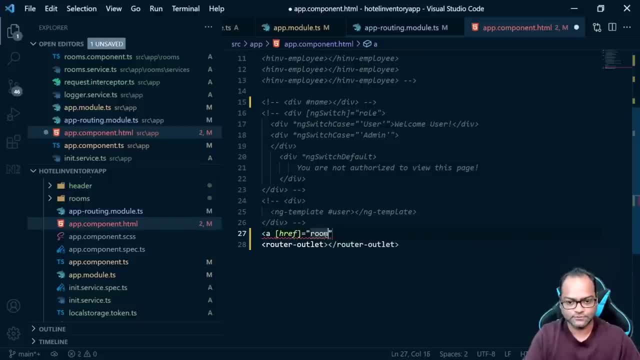 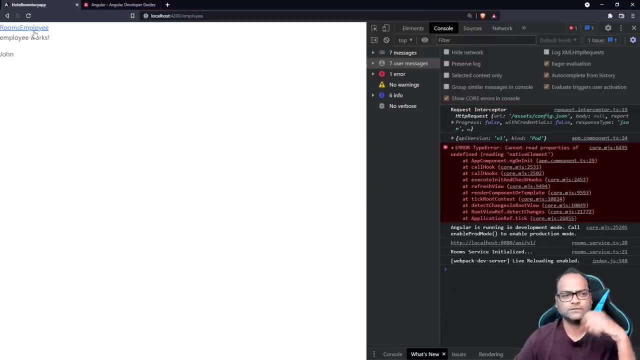 Of course we can do: href equals to rooms and I can say rooms And similarly I can say employee. So these are two anchor links which are available And let's see, let's click on employee and it works. Let's click on rooms. 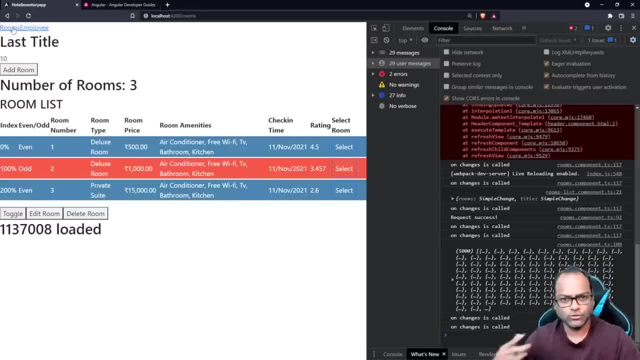 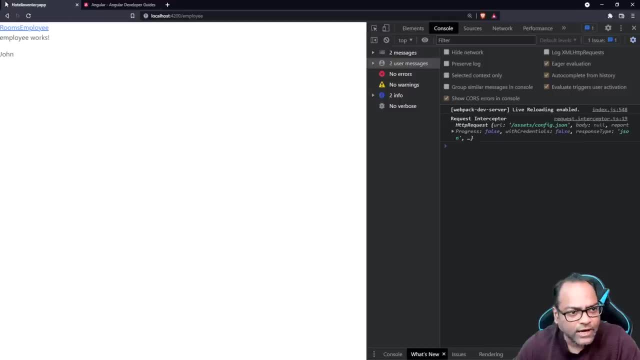 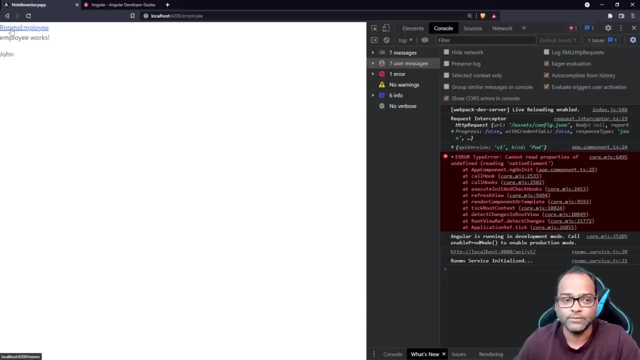 Then why I'm saying not to use href. Do you saw any odd behavior as we discussed about? Click on employee and you can see the entire page is getting reloaded. This is not an SPA, This is multi-page application. This is something which happens in MPA: multiple multi-page applications. 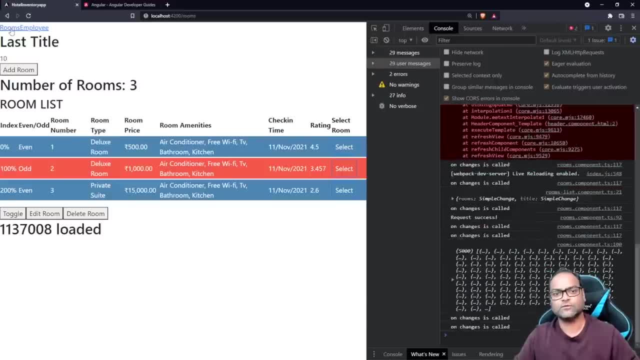 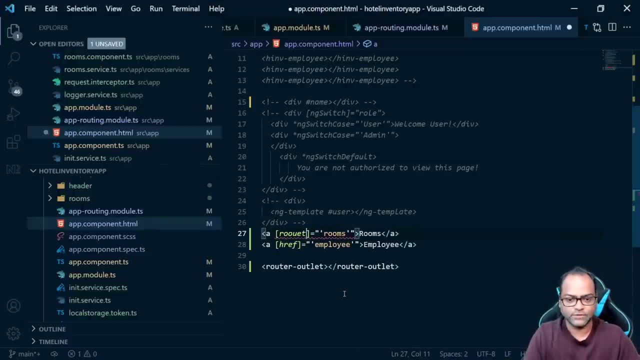 Okay, Okay. So to avoid this, what you should be doing is, rather than using href, Angular provides a property So you can say: uh, router link is equals to, and let's see, click on employee and it works. Click on rooms. 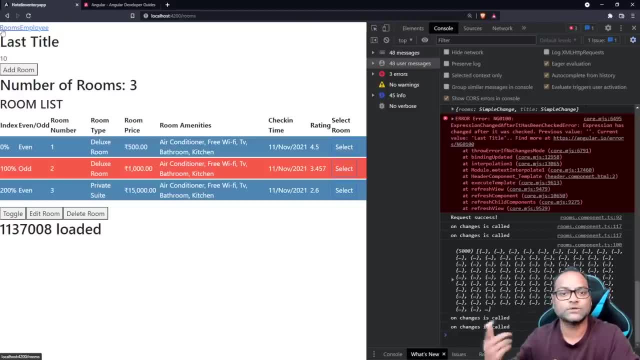 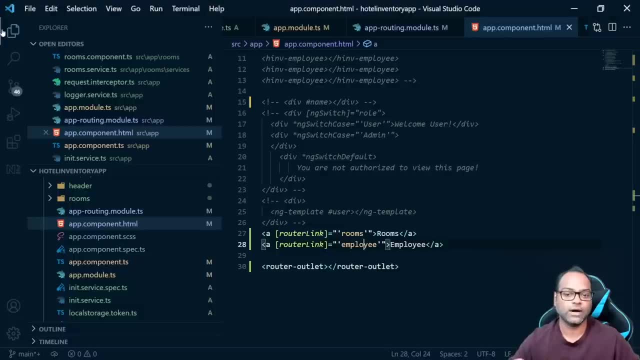 It works, But did you saw there is no page reload, So it means page is not getting reloaded. It's a single page application on the same page. The views are being changed. Now coming back to our this router outlet. We need to discuss it. 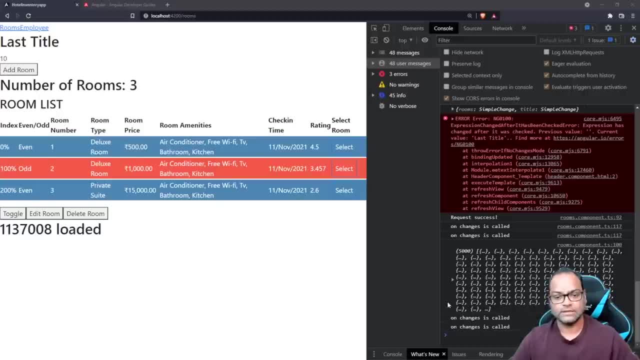 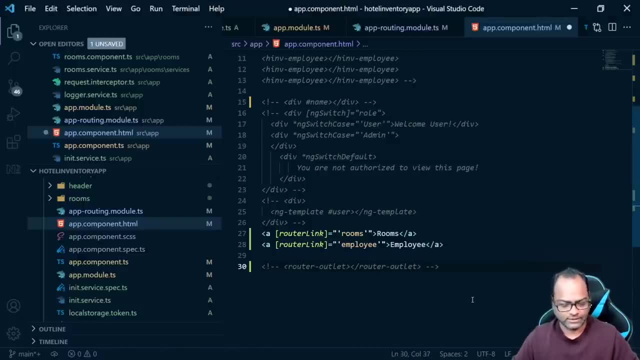 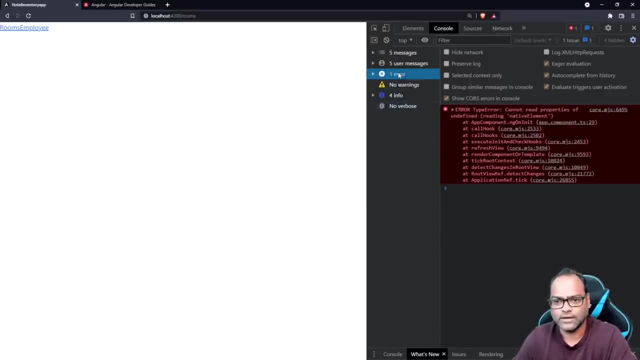 Otherwise how you will understand that how this works. So whenever you click on any URL, what happens? in case? I just keep this router link and remove this outlet. let's see, and nothing is getting loaded, So there is no error. You can see. cannot read out. 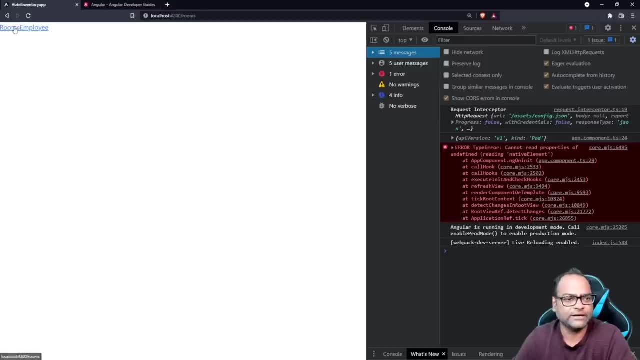 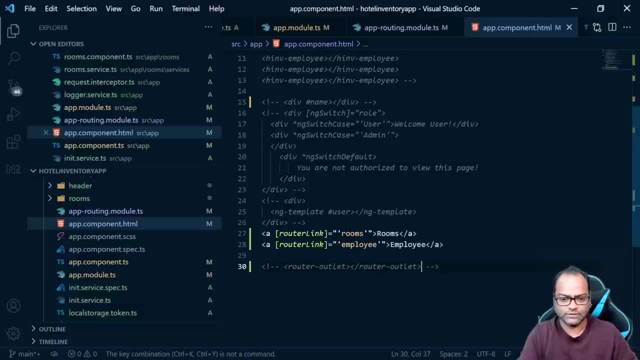 This is something which is ready. It's ready to earlier view, but there is nothing which is getting rendered. Click on rooms, click on employee: URL changes but there's nothing to render. So let's add back this router outlet and we'll talk about it. 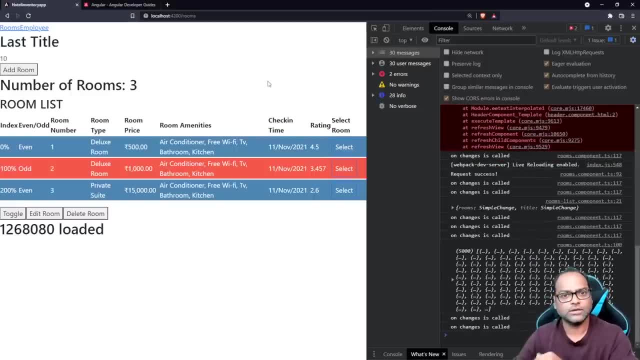 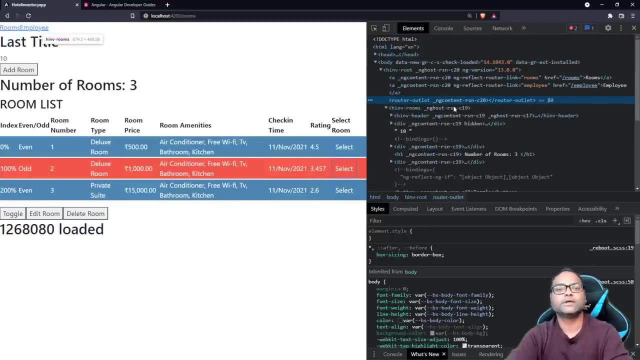 So whenever uh, that is any uh URL or you have some provided, some route which is configured, The thing is Angular looks for- let's go back to this. So Angular looks for this router outlet. on your view, If this router outlet is available, whatever component which you have configured here. 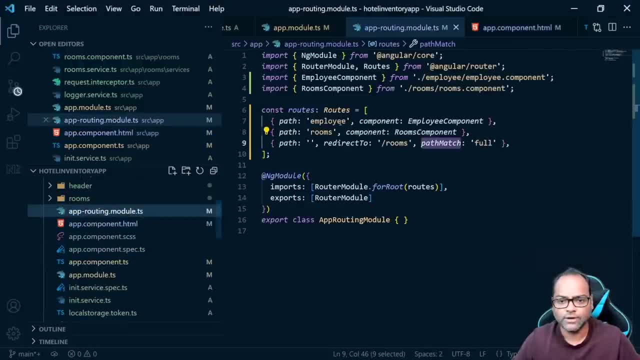 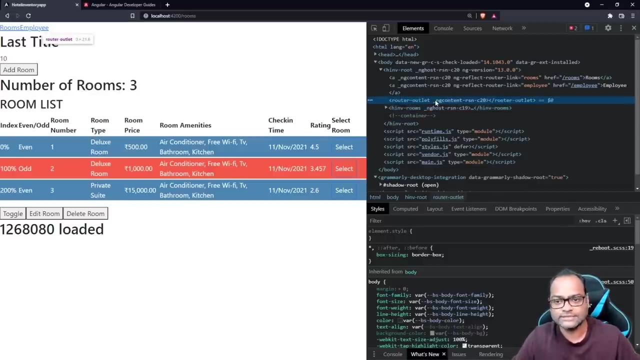 So let's go back to the configuration again. So here you have added some configuration, right, So load this component. load this component, So Angular will add this component just after this router outlet, remember this. So you have rooms added just after this router outlet, in case this router outlet does not. 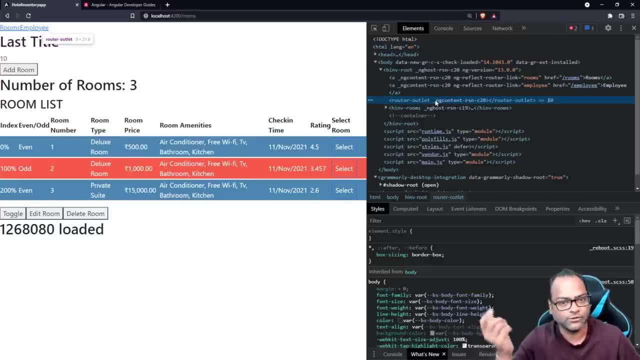 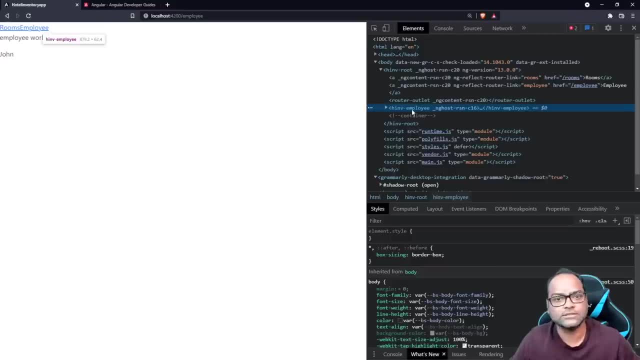 exist. I mean won't be able to add this because there is no router outlet. So same in case I click employee, it will just remove the existing component and add this employee component. This is how this works. This router out router functionality works. 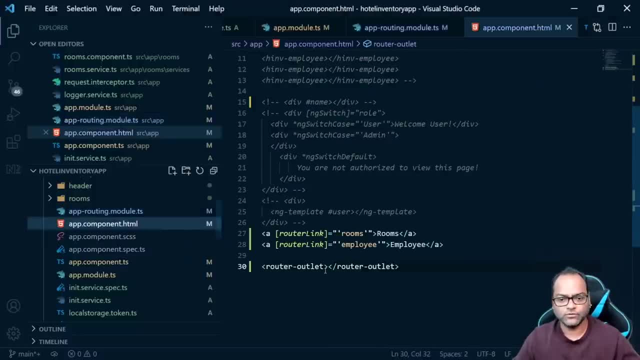 So make sure. I mean, uh, when you start you, it will happen that you will miss router outlet a lot. Even it happened with me And I still do that. I mean, whenever I'm doing a live coding I miss it generally. 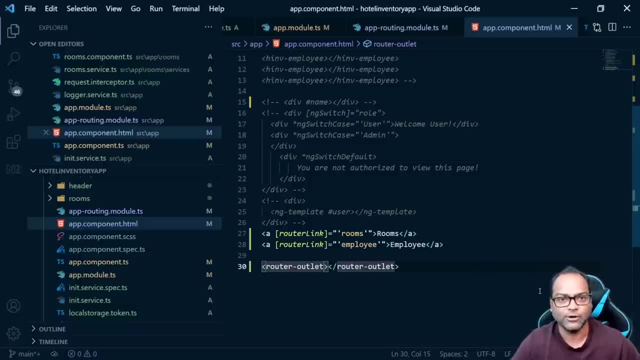 I mean not generally, but occasionally. not it doesn't happen A lot, but yes, it it happens. So, in case your router is not working, router functionality is not working, just check if you have router outlet available or not. 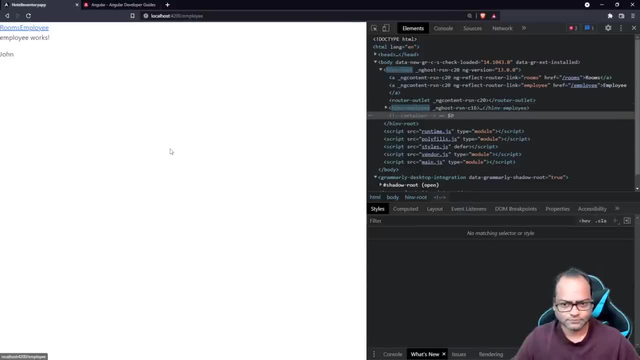 And that's it. It will be taken care of now. Now, what we have done: we have added, uh, the routing functionality. We have added the routes, We have added anchor links to shuffle between it. We have added the default route. we have, uh, even, yeah, that's it. 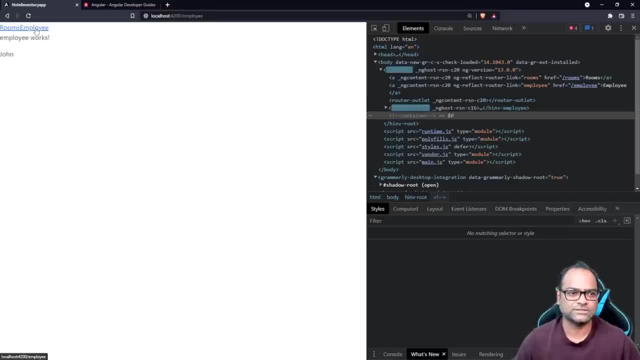 So now, what we will do is now, of course, this URL: Uh, this navigation doesn't look nice, right? I mean I, of course I'm not going to use this application if I have to. I mean, uh, 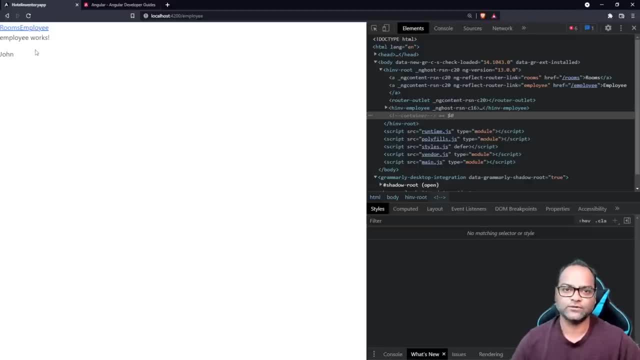 how does you? you, I looks like. so what we can do is let's go ahead and add material. next This video, we will be adding angular material to our application and we'll also add a navigation- nice navigation- using angular material itself. 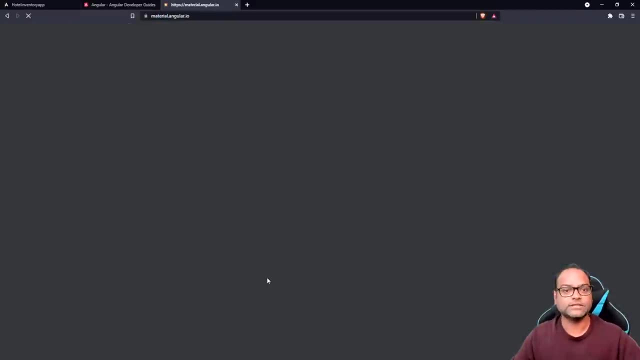 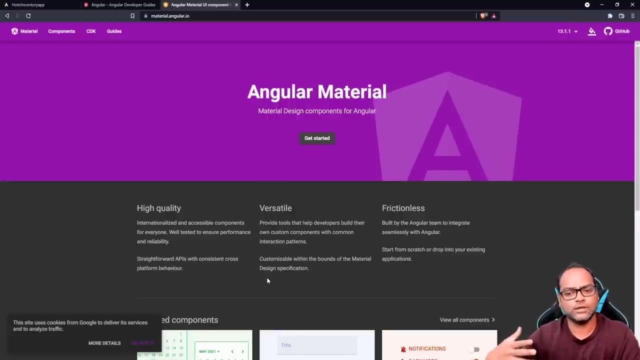 So, uh, the page is materialangulario. Okay, This is the webpage where you can read, uh, everything about angular material. So it's a uh, UI component, UI component library, similar to remember we tried to add. 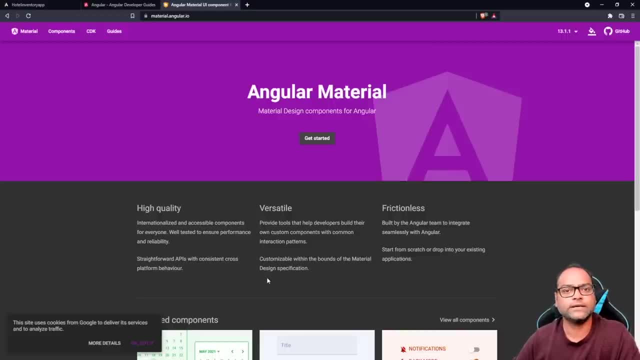 a angular bootstrap, So this is some similar, but it uses the material CSS, So material- or you can say it uses material design, So material design- is, of course, something which is, uh, created and maintained by Google itself, So they've created a component library on top of it. 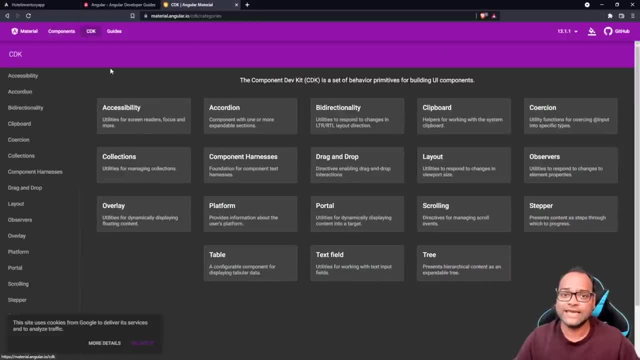 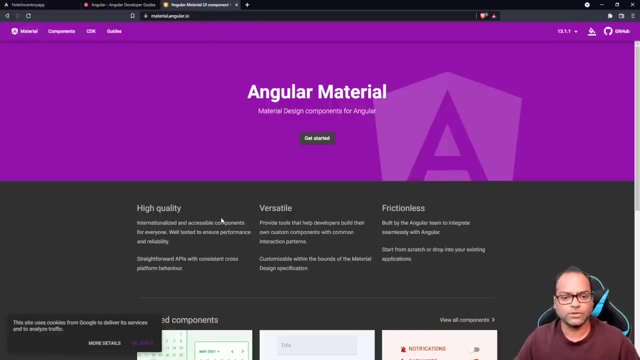 You can see it has a lot of components. You can go to components. It provides CDK as well, In case you want to build your own components, uh, which uh angular already has, and it has a guide, So let's go ahead and add this. 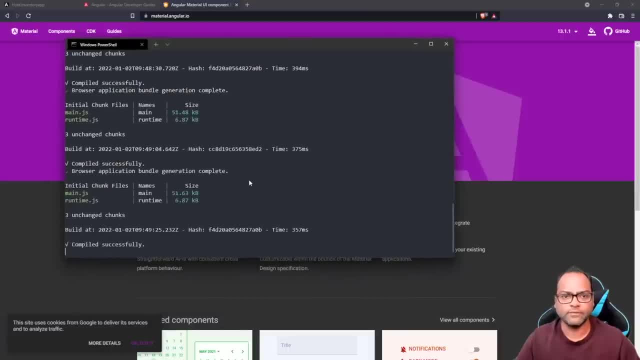 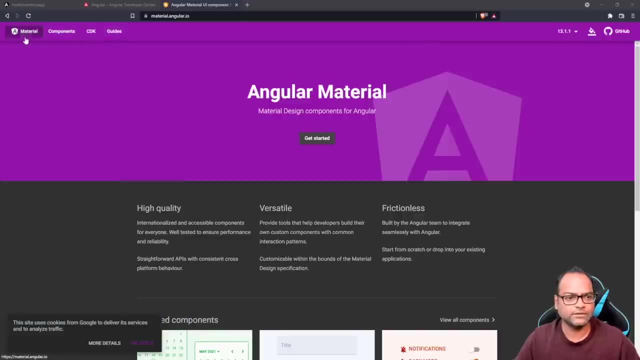 The first thing which I'm going to do is I'm going to stop the server because it will add some configurations to angularjson and I have to anyways restart it. So, uh, let's go ahead and get started. So it says: uh, there are some uh guide for angular and guide. 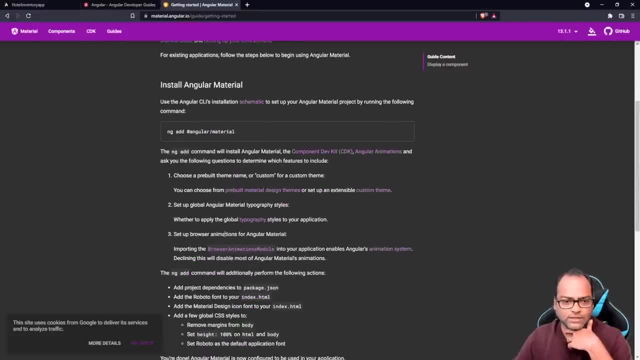 So let's go ahead and get started. So it says, uh, there are some uh guide for angular and guide Okay, And then there are some steps which we have to do. So the easiest thing or easiest way to install angular material is just to run this command. 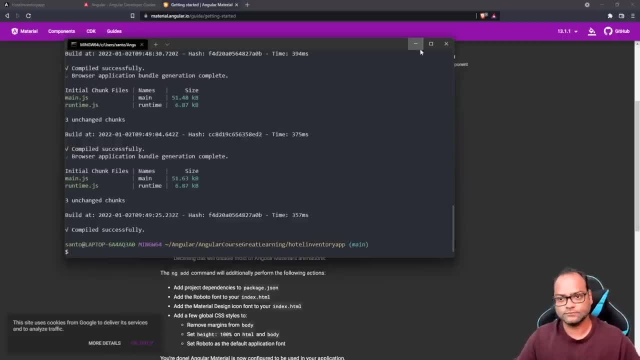 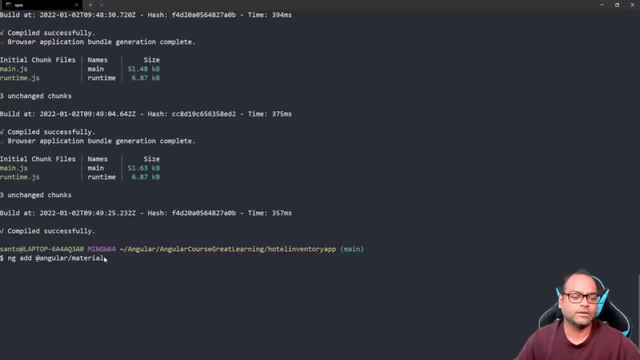 So let's do that. So ng add angular slash material. So it says the angular material 13.1.1 will be installed. I would say yes, Yes, I'm looking at, I'm using angular 13.. And it will ask you to choose themes. 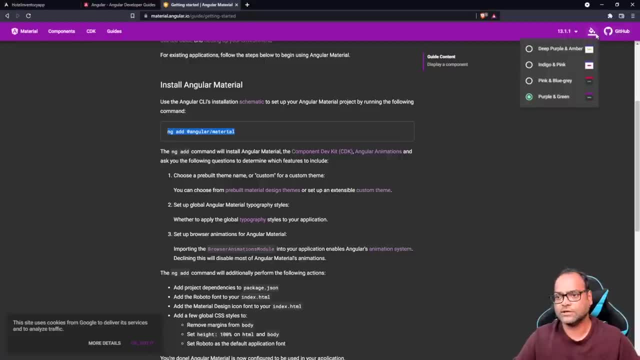 So the themes are same. which is available here. So you can see, uh, it has purple and green, pink and blue, deep purple and amber, And it will ask you to choose themes. So the themes are same. which is available here. 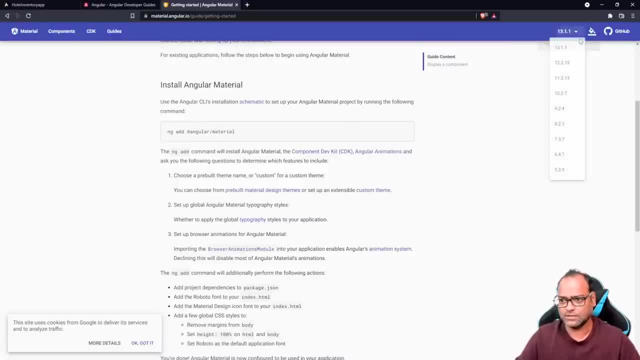 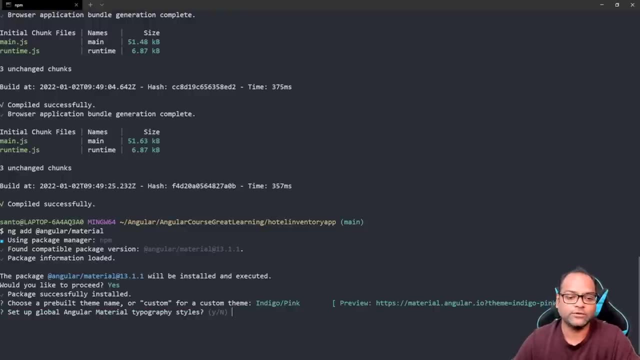 So the themes are same which is available here. So the themes are same which is available here, And you can choose whatever you like. So let's go with Indigo and pink, which is the default. You want to use angular typography. 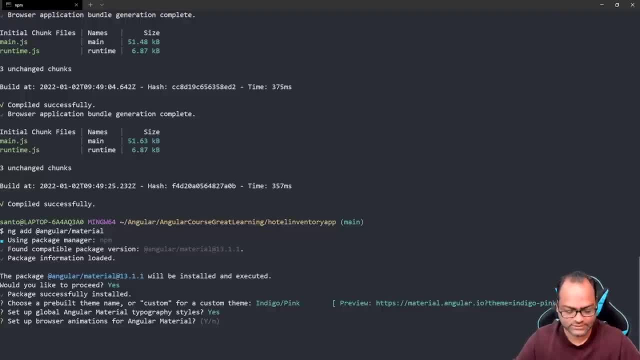 We are not going to use it, but it's added. Do we need animation? Yes, we need animation because a lot of angular material component uses animation. You can disable them if you want to. I mean in case you are using some older browser. 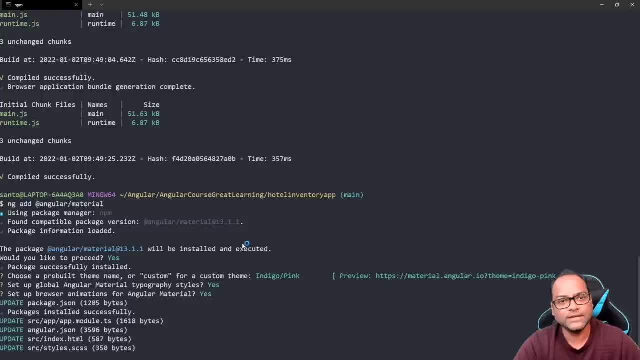 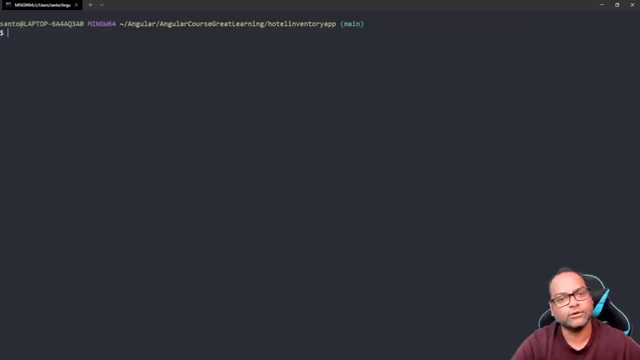 We have seen, Uh, the animation doesn't work properly on an i11,. uh, in case you are, uh supporting it, If you're not supporting it, you're lucky. Now, uh, angular has itself dropped the support for i11 and most of the uh, most of the applications. 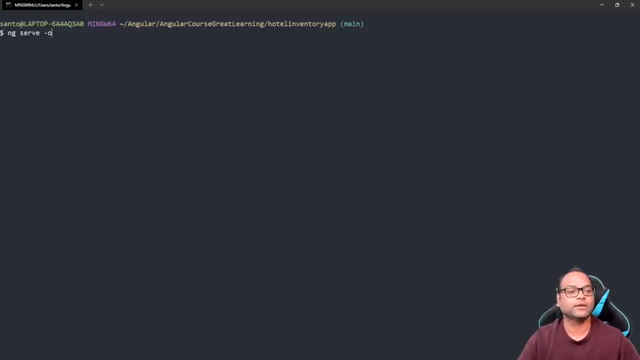 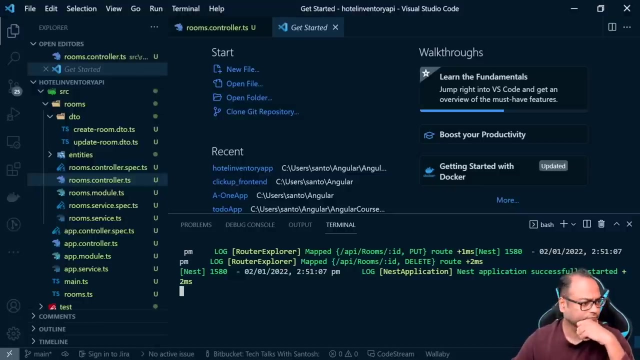 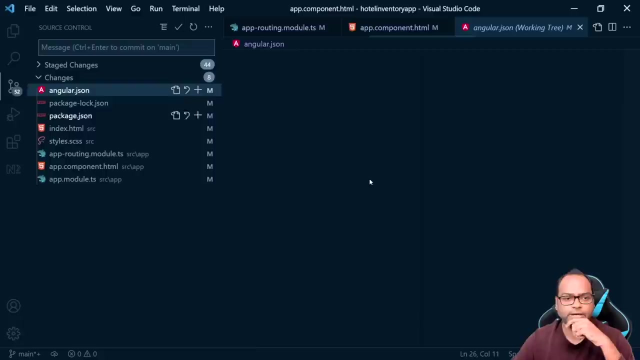 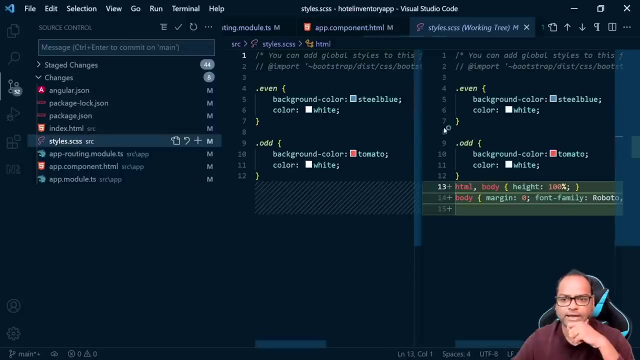 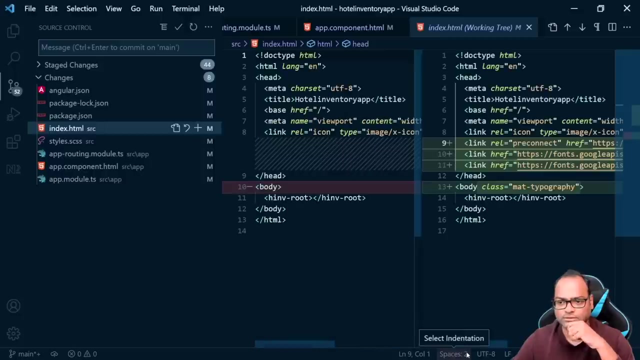 out there doesn't support i11 anymore And now it is added, Let's go ahead and see the changes. Okay, So it adds this uh CSS. you can see the CSS is added here and it will add some styles. It added some meta tags here and link uh, which is which is to you: uh load material. 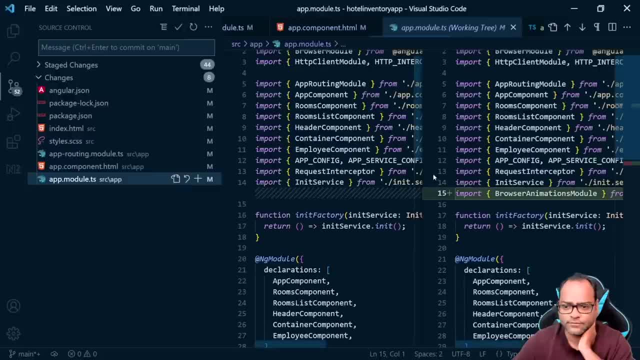 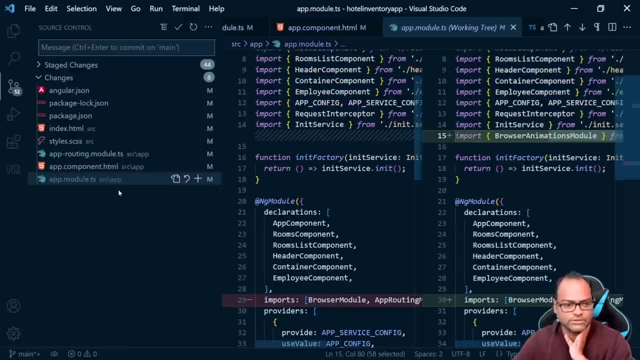 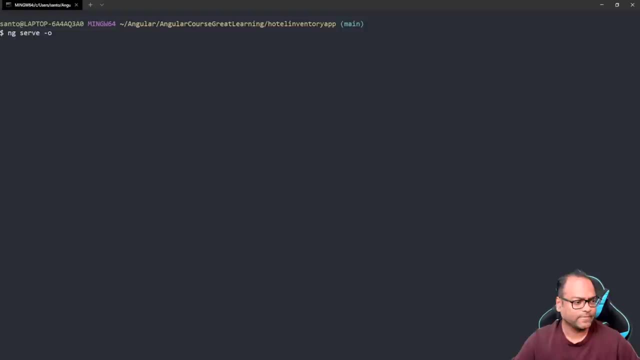 icons, And it will also add browser animation, because we said we want to use browser Any. uh sorry, We want to support animation. So this browser animation module is added and that's it. Let's go ahead and run our application and see how it looks like. 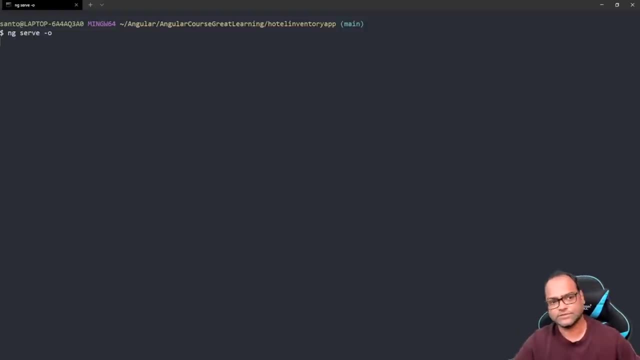 Remember, we have not added the uh navigation as of now. We'll do that next Once we see, uh the changes on our application. Okay, So, Okay, Okay, Okay, So, Okay, So Okay. 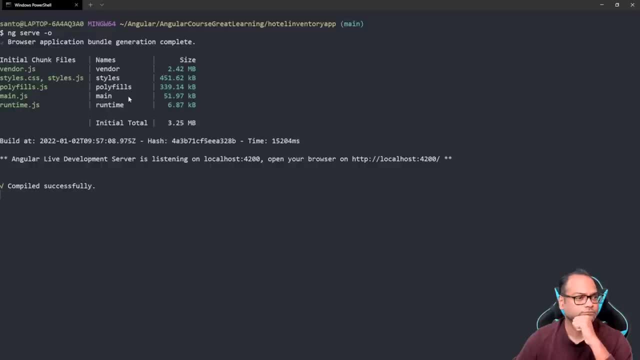 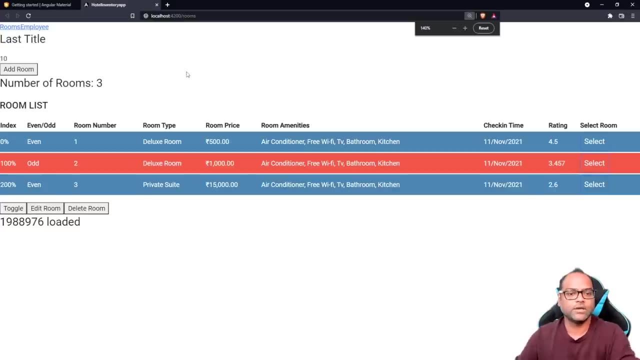 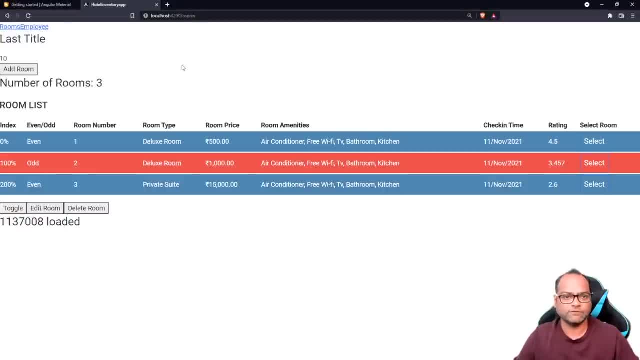 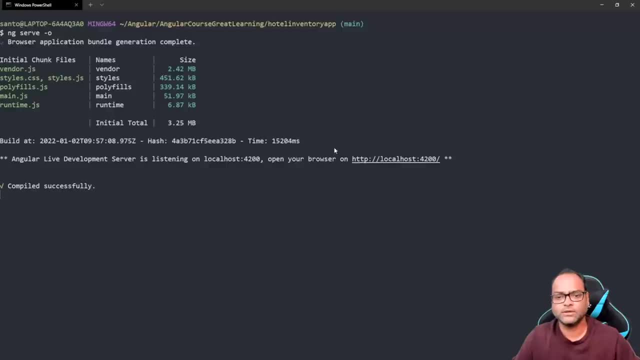 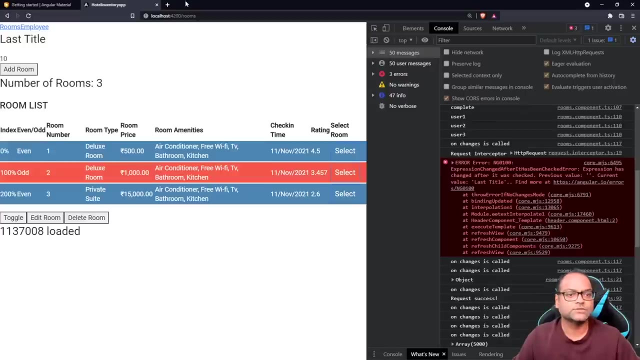 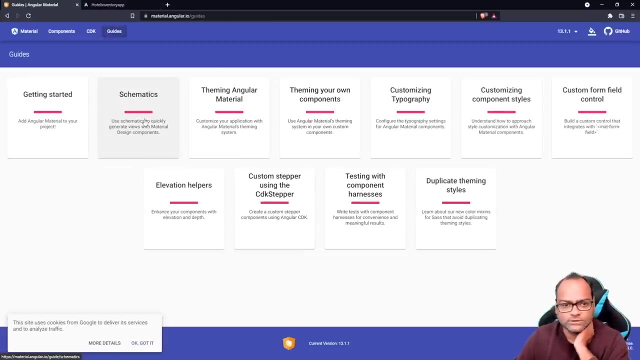 Now click on employee rooms. Everything works. So Let's go ahead and add the navigation option to the internet on the left. Okay, So let's go back. Uh, So go back to it, Okay, Okay, Okay. So, unfortunately with this part, so let's go ahead and check homepage and timer icon. 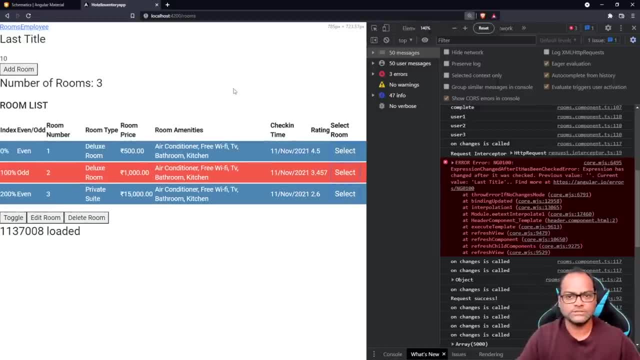 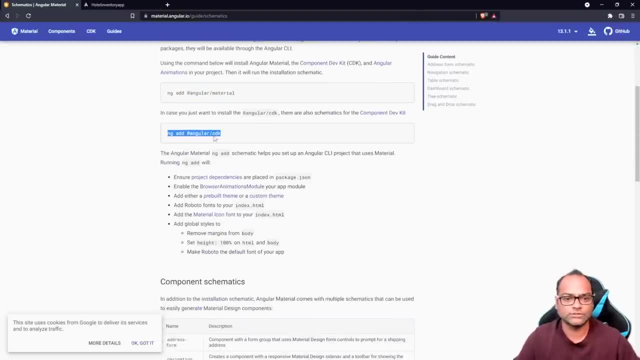 on the right for every setting option. just refer the docs so you can see. uh, this step is available here. and in case you want to install cdk, which we don't need as of now, we what we want to do is we want to create a navigation, so for 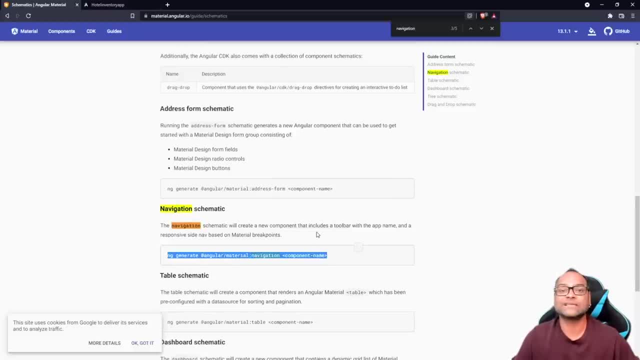 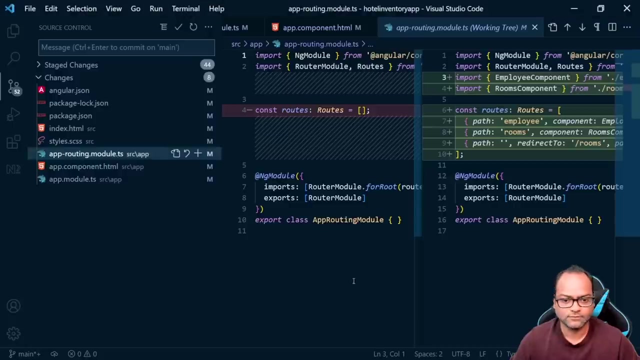 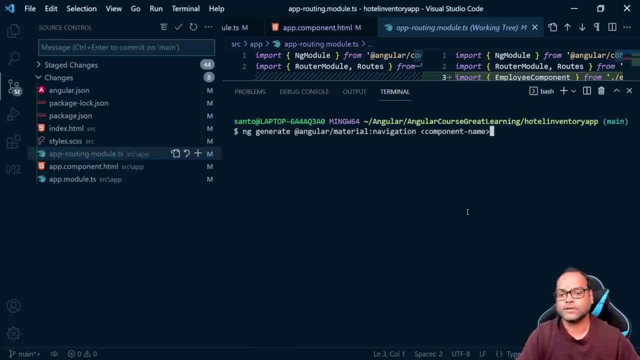 creating a navigation. there is a navigation schematic which is available. it means it's a command which will generate the entire navigation page for us and we can just use it. so let's go ahead and do that. i'll start here, so i'll say: this is navigation, so i'll call it as this is, a app nav. 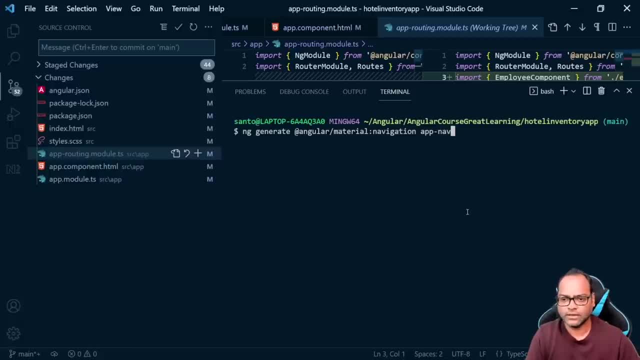 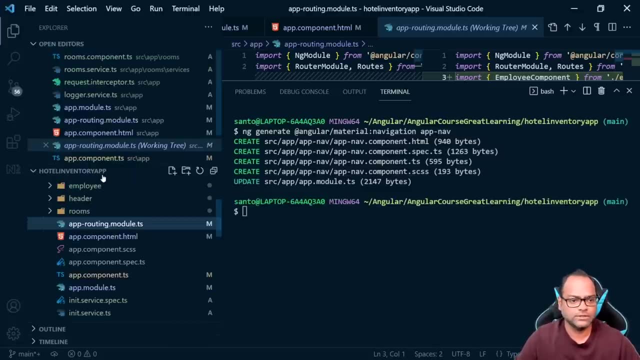 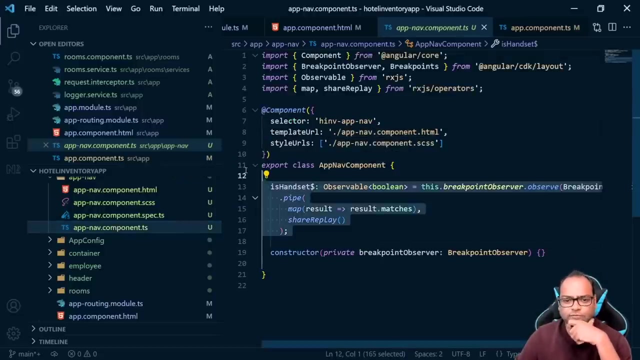 app navigation and this is done. so we have uh, this app nav, or we could have just said: navigation, that's, that's also fine, but yeah, so we have this uh component available here. let me just close this, and it has some already code which is available so we can see: okay, this is available here as well and some breakpoint observer. i mean this is. 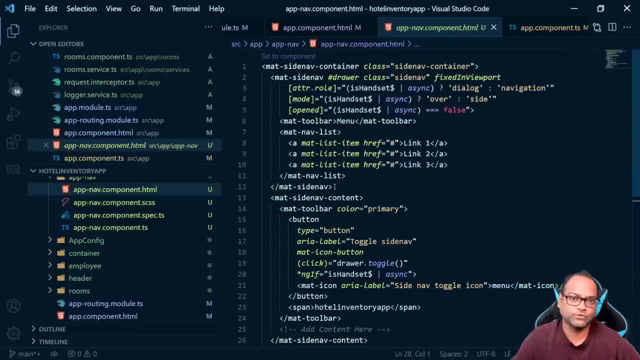 something which you may have to do by your own in case you don't use the schematic. so let's see how it looks like. so what i'm going to do is: uh, you can see, uh. yeah, uh, you can, you can see, uh. it has some uh, matte list, some with some href we will be replacing. 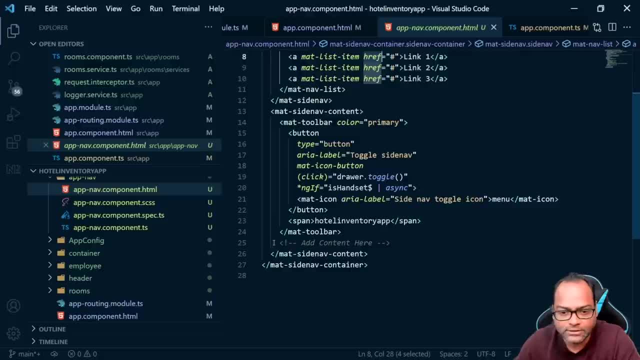 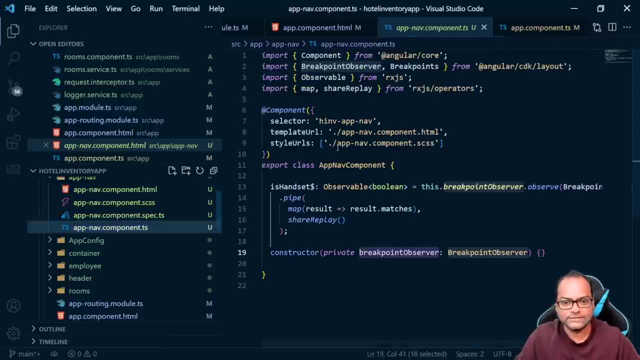 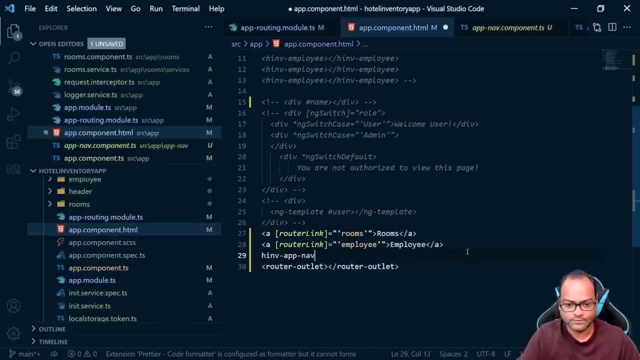 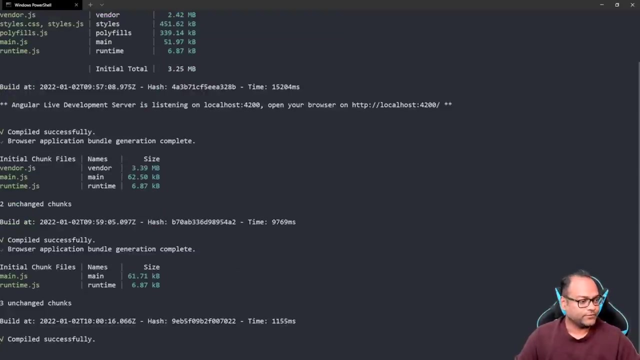 these hrefs with router, router link, and this is where the content goes. you can see it says add content here. so, uh, let's replace and make this component available here. let's comment this out, let's comment this and let's see our view. let's see our application. so you can see it has some menu link one, link two. 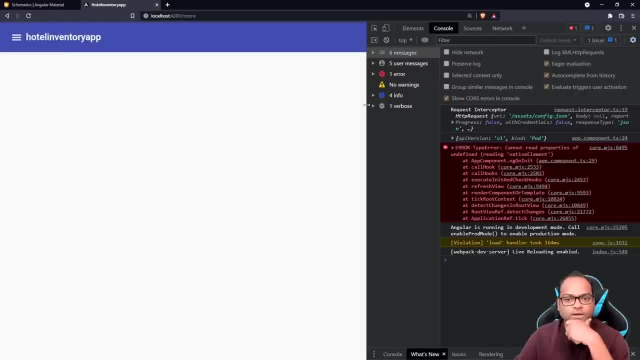 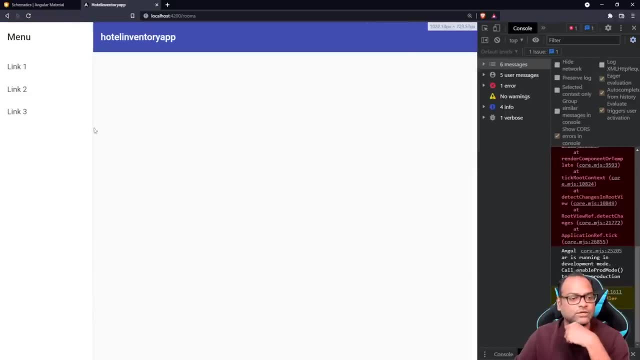 which, of course, doesn't work right now because there is nothing which is configured. but you can see also, this is responsive, so you don't have to actually go ahead and, uh, make this responsive. you don't have to write any extra css, this is all taken care of. so a responsive navigation bar created for us without 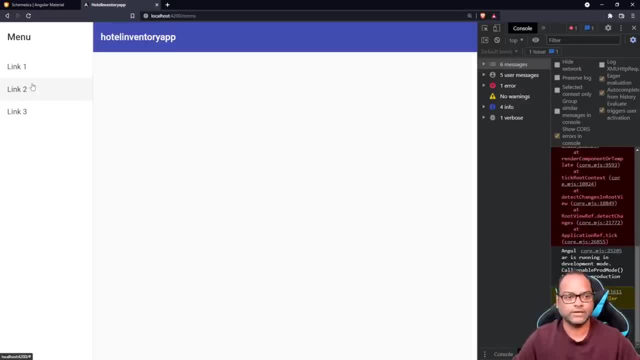 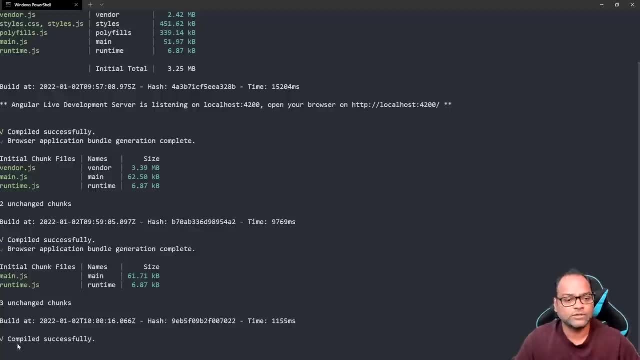 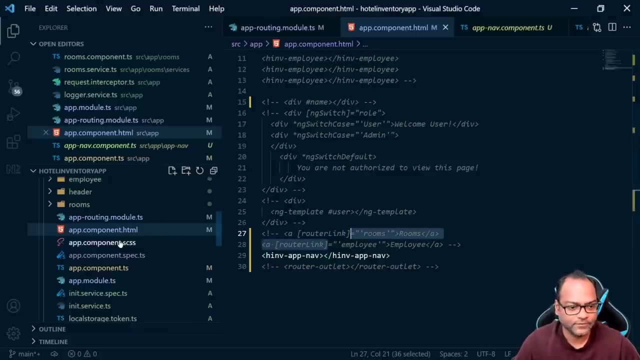 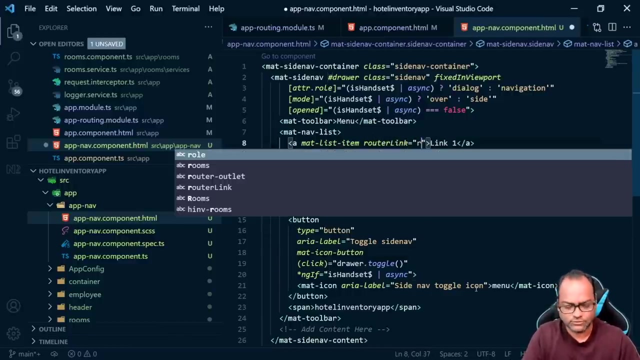 even writing a single line of code. yes, this is what angular material does, or this is how you can actually utilize the schematics which is available by angular material. so let's uh, add some. let's make this navigation work. so here let's go back and we said: here we'll add router link and, as we already know the routes, we don't. 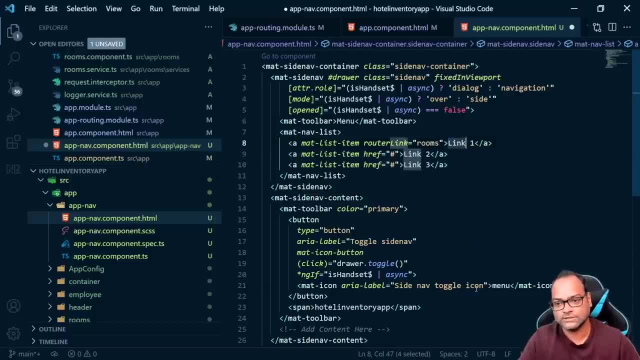 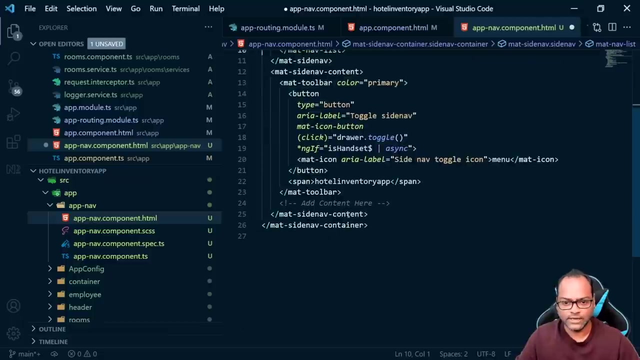 have to actually go ahead and move it in box so i can say, okay, this is uh rooms and this is a router. link is equals to: i'll say: this is employee and this is a native application source component. we'll say this is employee, remove this. and now we uh want to add. 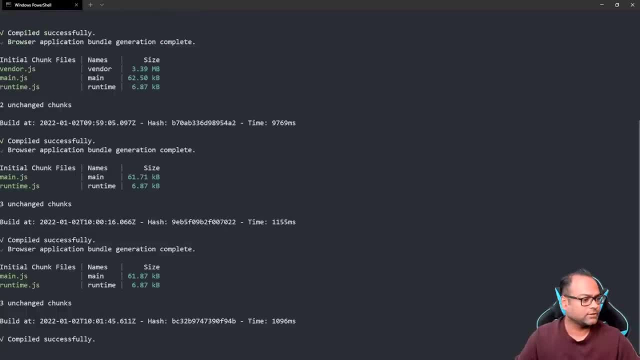 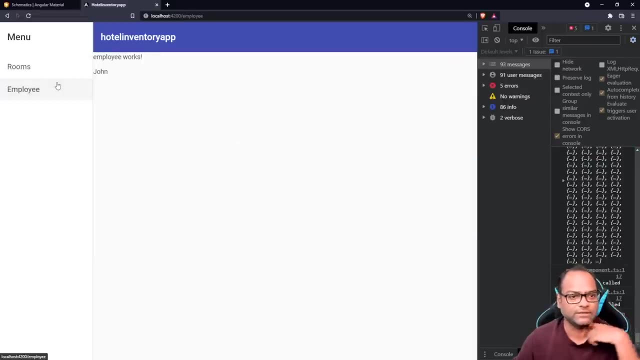 a component here- router, outlet- and let's see our application networks right, so you can now navigate to rooms, you can navigate to employees and everything works fine. so this is how you can uh add angular material to our application, uh, or any application. and another way you can do this is when you gain more options, for example for variant. 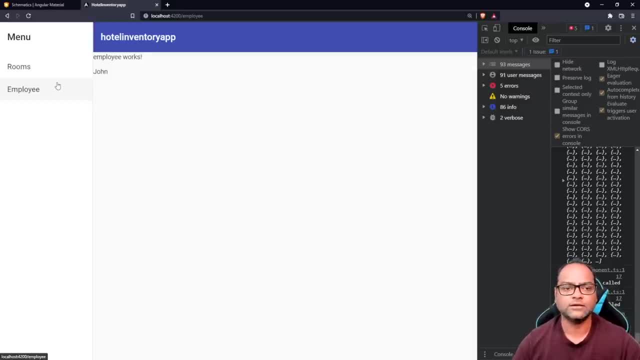 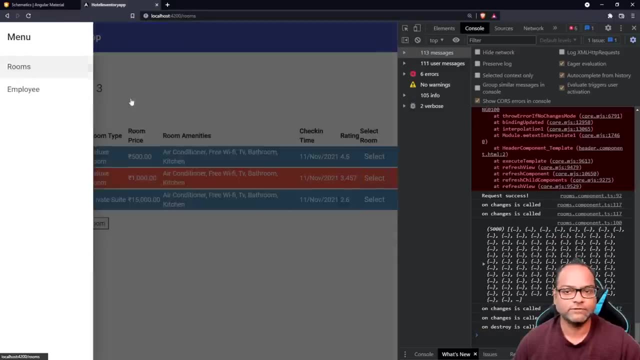 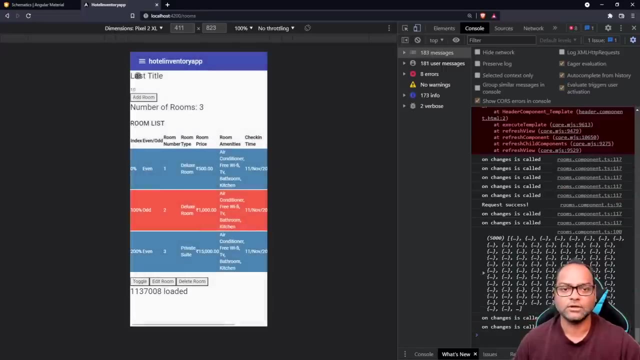 And you can also configure the routes And you can also add navigation without making much of an effort. So you can see it is responsive, It will work for mobile, So you can just click on mobile here and it will work, So you can move to whatever URL or whatever routes you have configured. 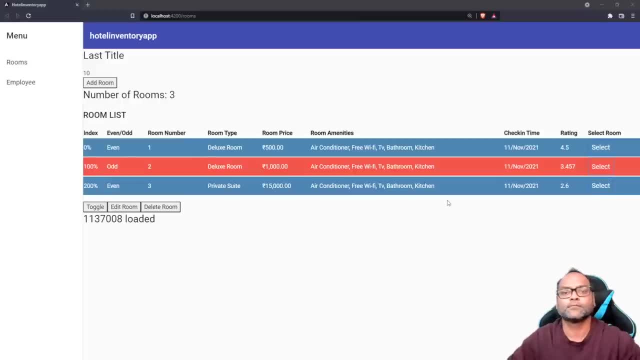 So this is it from this particular video. So far, what we have done is we have configured the route. We also saw how we can set default route for our application. But let's see, there is one problem with whatever we have done so far. 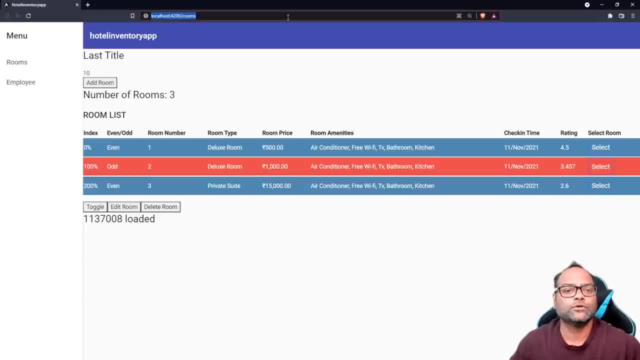 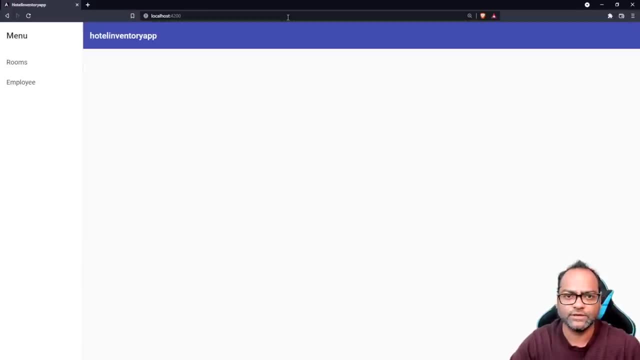 And we will see how we can fix it. So here, let's say, if I try to enter a route which does not exist- And this is where the problem is- You can see blank page. And now, if I go to the console log, let's see something interesting there. 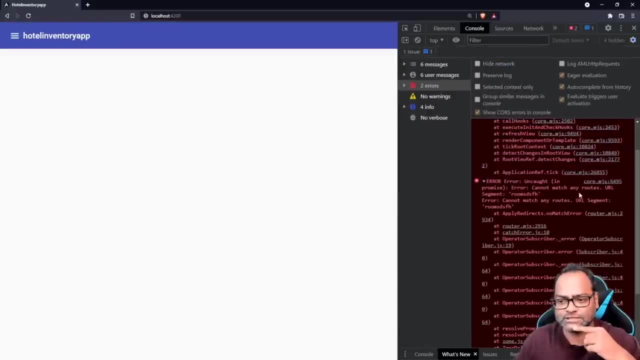 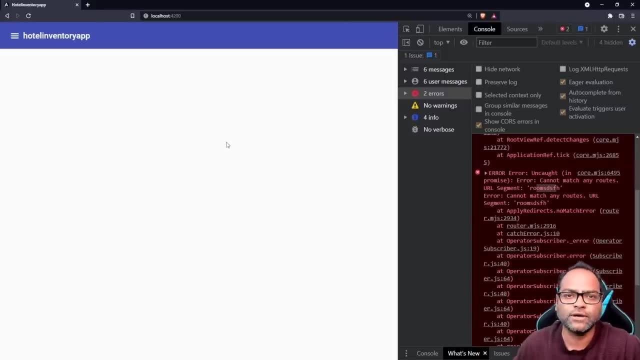 So in console you will see an error which says: cannot match any routes with this particular. So let me just zoom in. And of course this URL does not exist. but we should not give a blank page Right What we generally do in real time applications. you might have visited a lot. 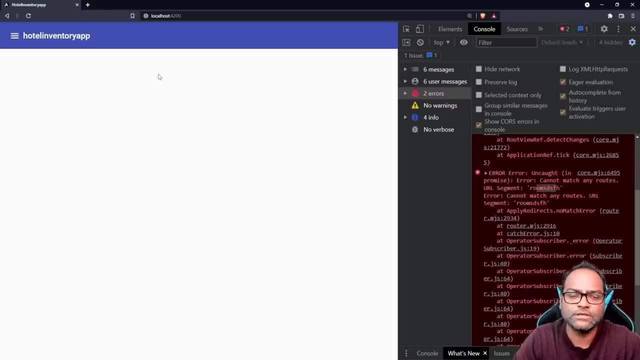 of applications. you might have used it. a lot of web apps, What you generally do. Yes, the answer is 404 pages, Right, In case you guess that you are absolutely right. So the solution is to add a 404 route. 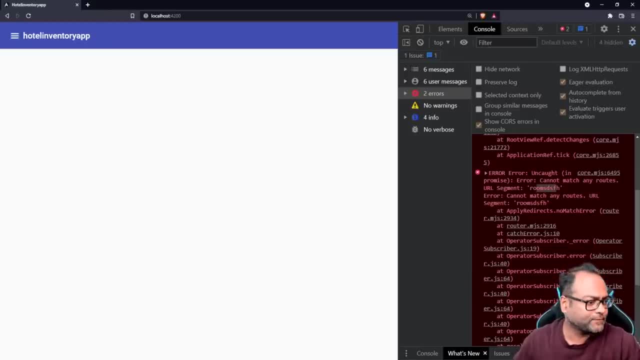 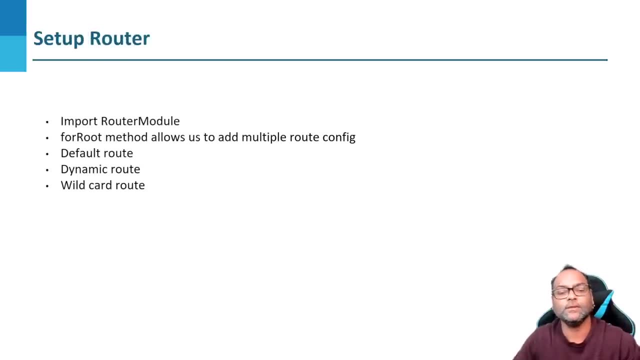 How we can do that using Angular. So this is where We are going to do. So this is where we are going to do a wildcard route example, or we are going to see an wildcard route example. So let's go back to. 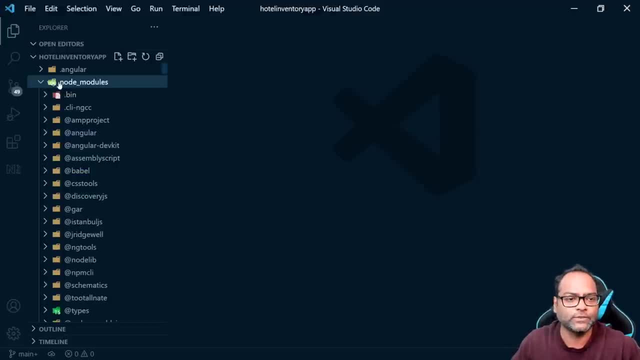 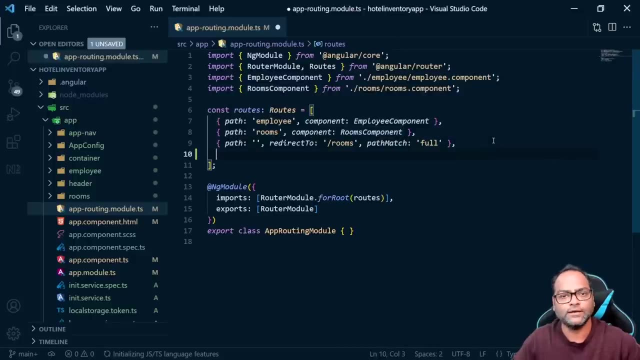 Let's go back to our code and let's open the configuration file. If you remember, it was app routing module and we had added this default route. Now let's go ahead and add a wildcard route, which will take care Of and we'll talk about it. 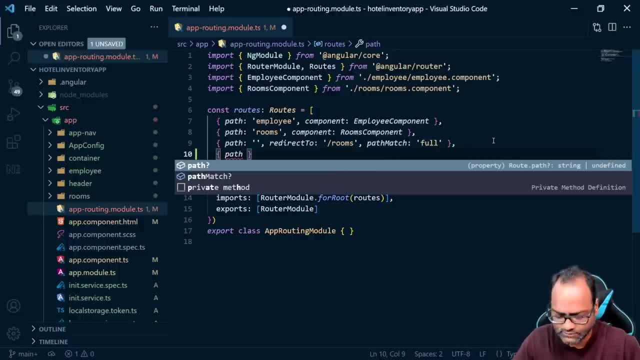 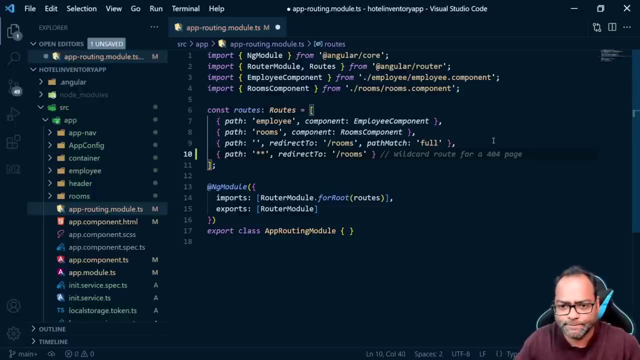 Let's first add it. So how do I add wildcard route? You have to say path and you will say double star, which is: Let's write this and talk about it. Yeah, So the path double star says any route which does not match to any. 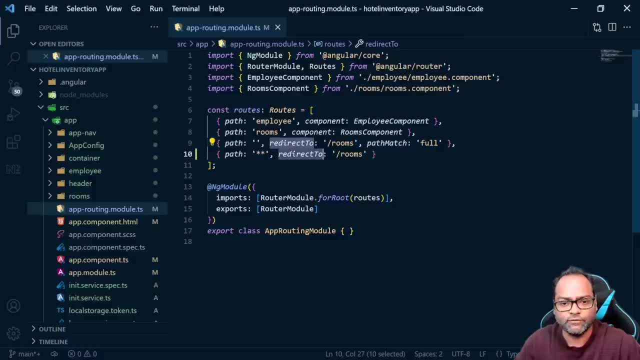 of this will be captured by this, And what we are doing is we are redirecting to rooms. Do we need to? The answer is no, We don't. So let's create a four four page and let's redirect the users to four four page. 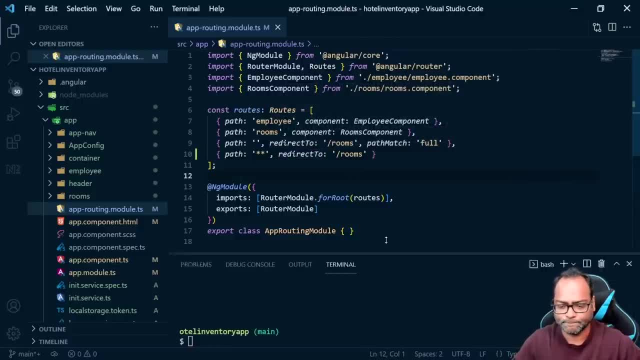 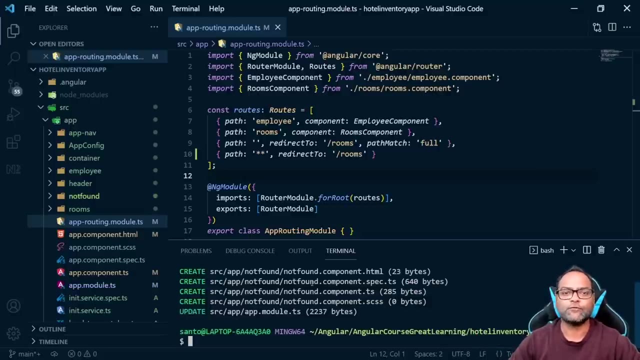 So let's add a component and we'll say NGC and we'll say: this is not fun, You can show whatever you want to. probably have seen a lot of uh inventive, uh ways to actually show not fun page. There are different applications which uses some uh, SVG, SVG. 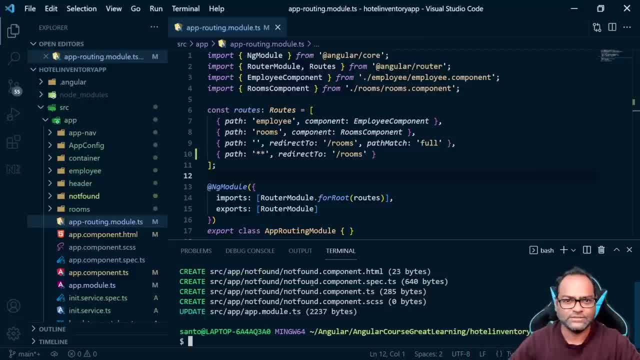 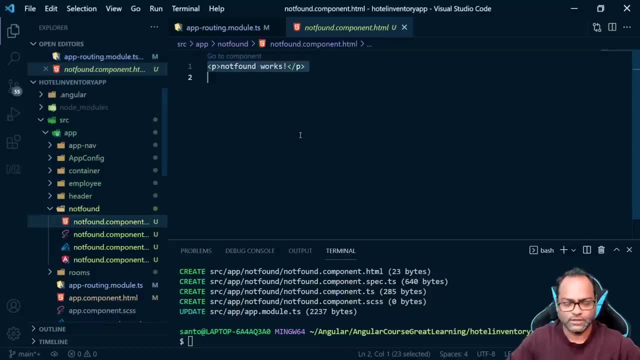 Like some skull logo. it depends, right. So whatever, whatever your use cases. So here we are adding not fun page and let's go back to component and I'll say this: or we can set the resource you are looking for does not exist. 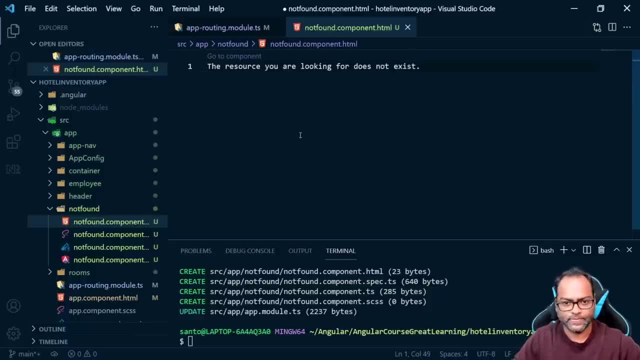 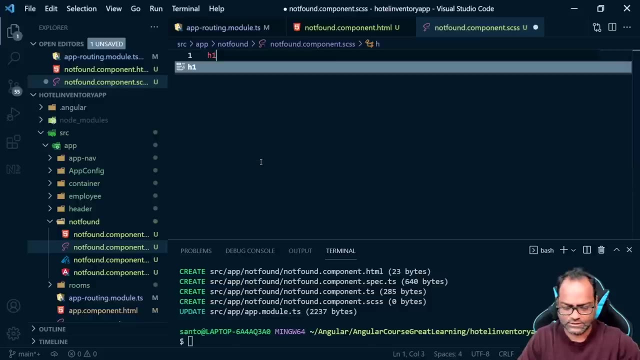 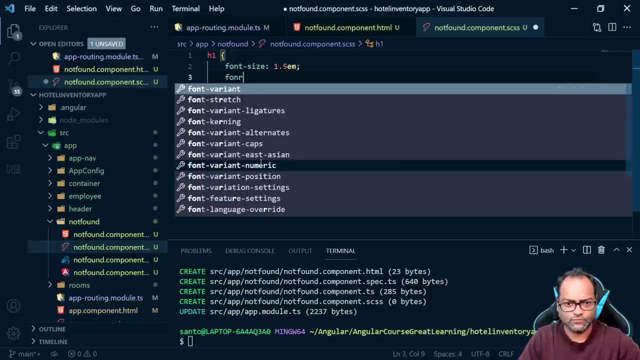 Right, So we can show this, and what we can do is we can, We can just wrap it inside a div and let's do just add some CSS, CSS here, That's fun. And we'll say: this is a font, So is then on color. 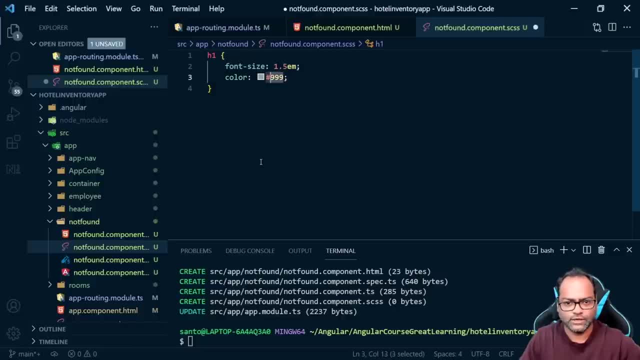 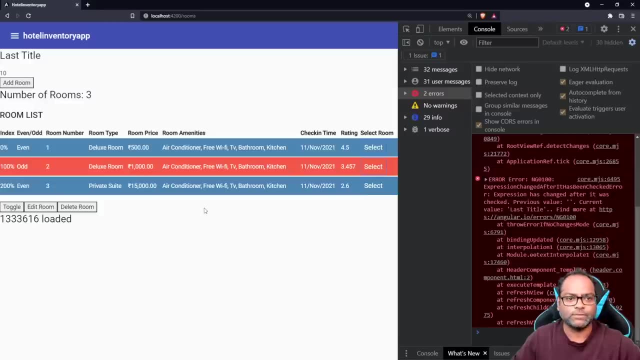 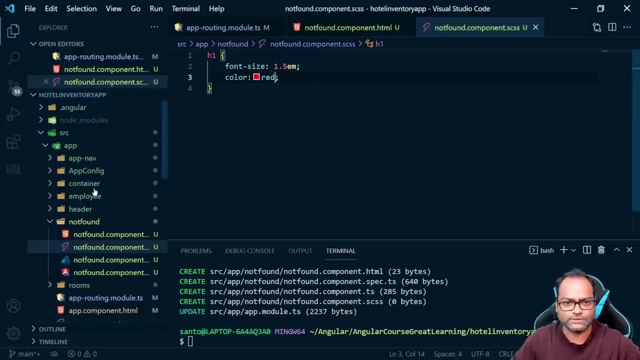 Uh, so color would do and we'll say: this is red. Let's see. let's go back To our application and let's try to enter uh URL. Uh, but again sorry. Um, right now it will be redirected to rooms, because we said it should. 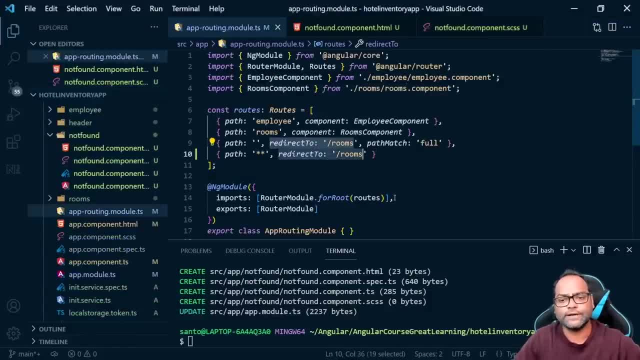 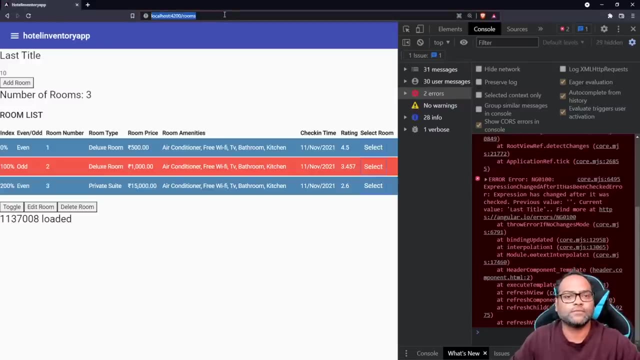 be redirected to rooms here, But what we want to do is we want to redirect to- of course of not- fun page. So we can say component and we'll say not Formed component. Let's say and let's try to enter URL which does not exist. 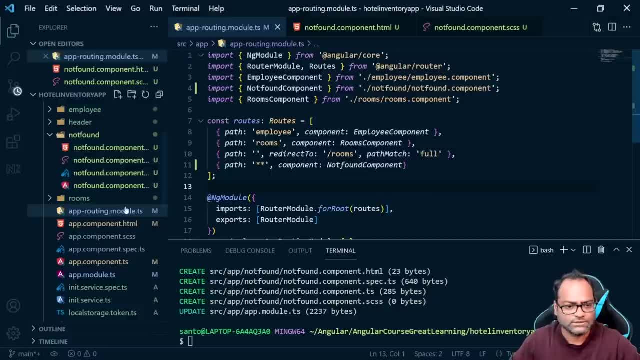 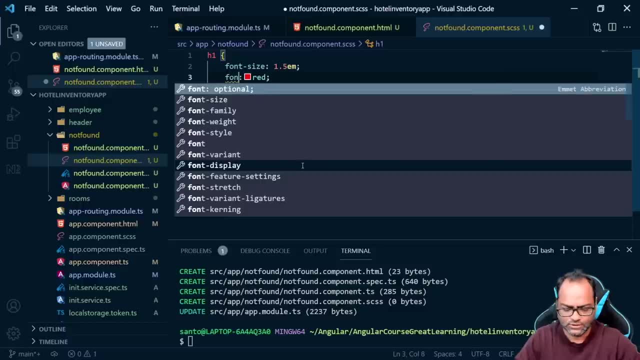 And here, Yeah, So the resource you're looking for does not exist. I think there is some problem with CSS, which is not taking the color. Probably should be font color. If I'm not wrong, there is nothing called font color. 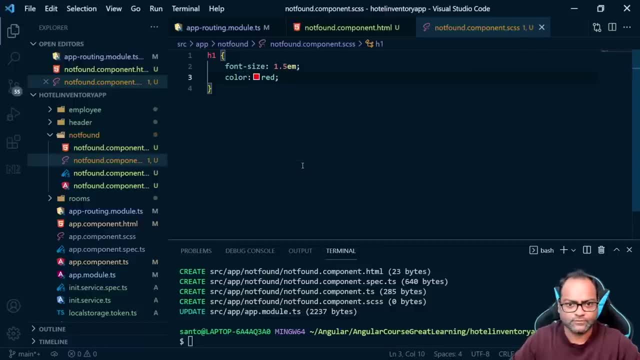 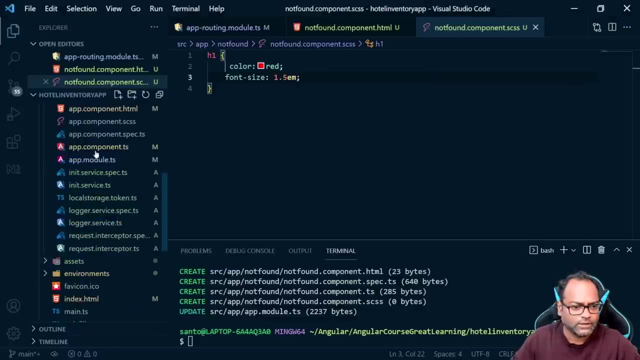 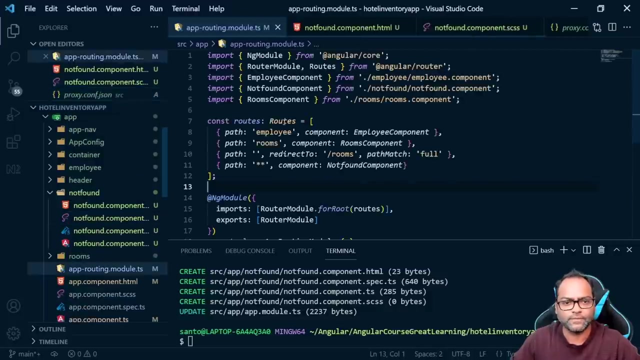 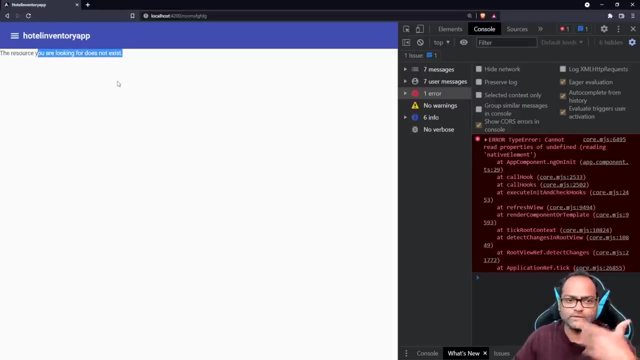 Hmm, That's strange. That's fine. So Okay, There is something wrong, but yeah, anyways, this is not what you want to do, So Yeah, So uh. now what we have is we have a four page which is available for us by using the wildcard route match. 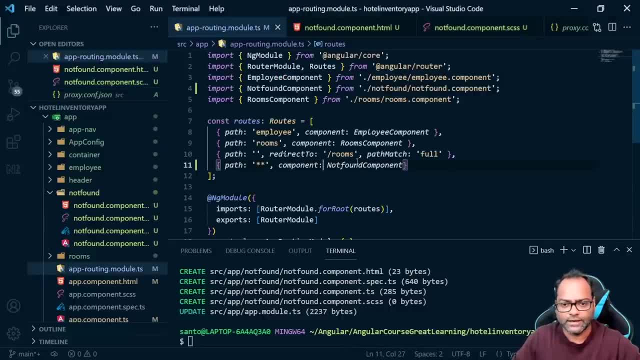 So this is how we can uh handle those scenarios, and let's see what's next. So now we will talk about how we can Create dynamic URLs. that is interesting, right? So what in case? I want to uh redirect a user to, let's say, room slash ID, right? 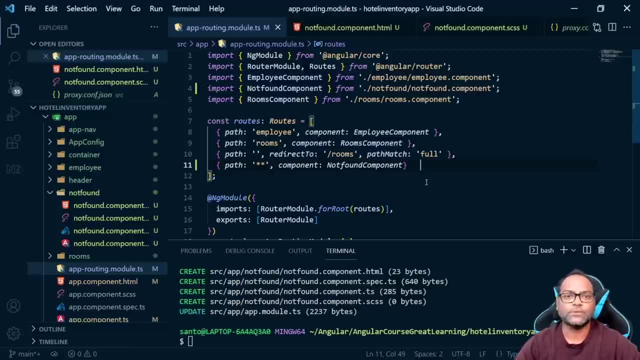 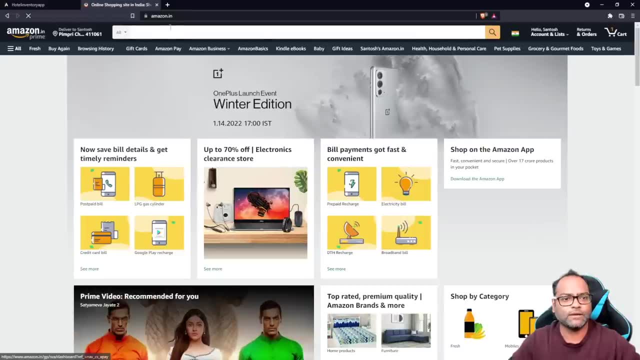 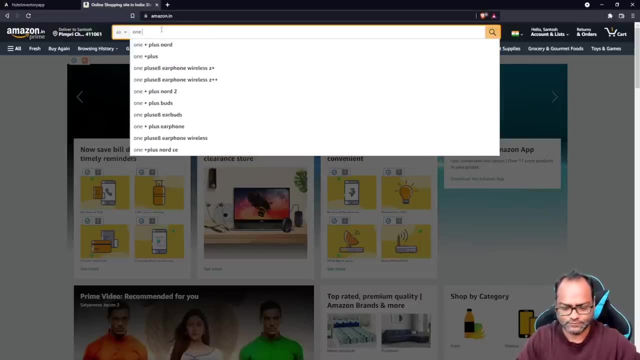 So it uh. you might have seen some, uh, e-commerce applications, and let's take an example of e-commerce application. Let's open one. So let's go to Amazon and let's click on, let's see any product. So I say yeah, one plus nine. 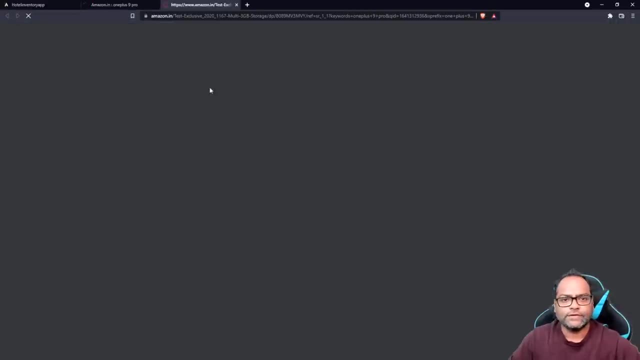 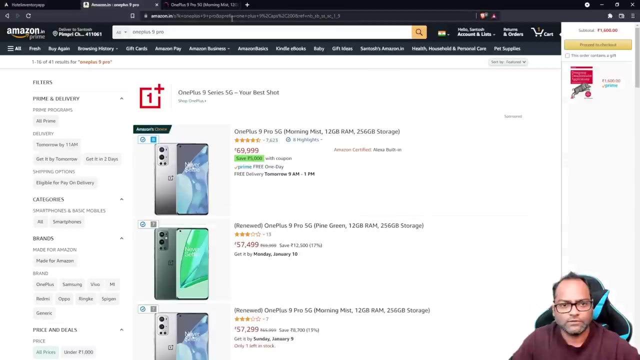 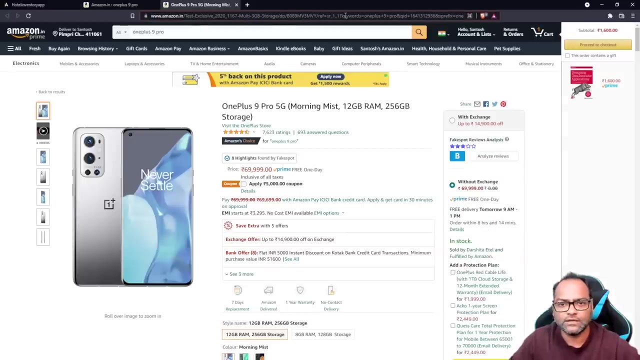 So, and when you click on this, you can see, uh, there are some parameters which is added after this, right, If you see this one, it has like S K one plus whatever your product name is, And after that, uh, you will see here. uh, you have keyword one plus nine pro equals to this lot of parameters which is added in the URL. 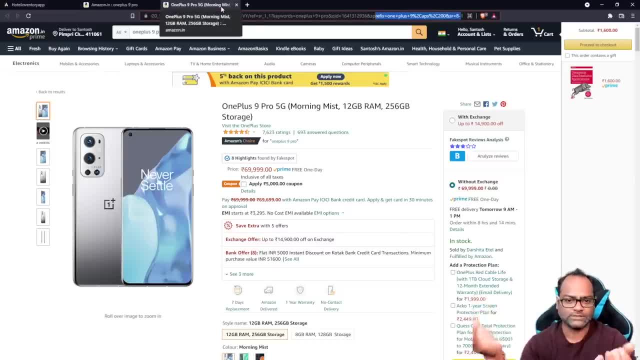 What in case we want to create some URL where we can pass some- let's say in our case, a room ID, And it opens a new page, right, I mean, it redirects to a new page. Let's see how we can do that. 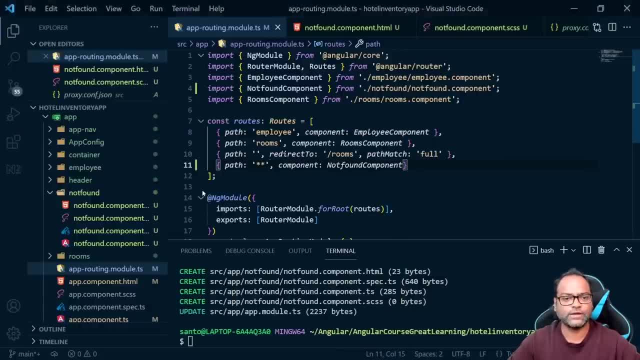 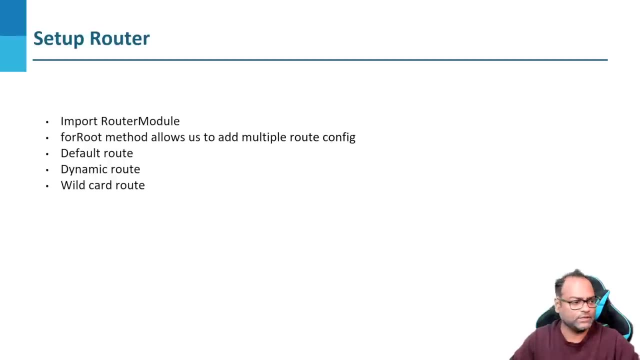 How we can configure a URL like that. So this is where we will be discussing about the concept of dynamic routes. We'll see how we can create dynamic routes. The first thing which we'll do is we'll go to room rooms. Uh, let's see the UI first. 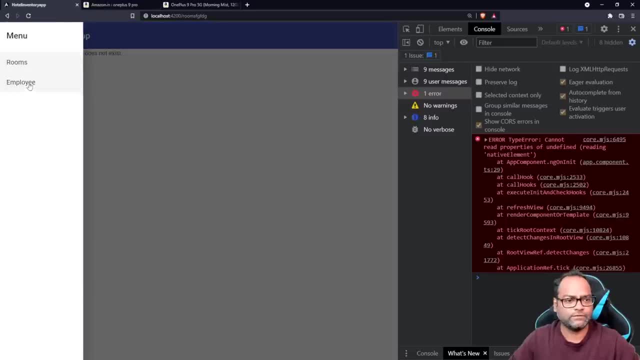 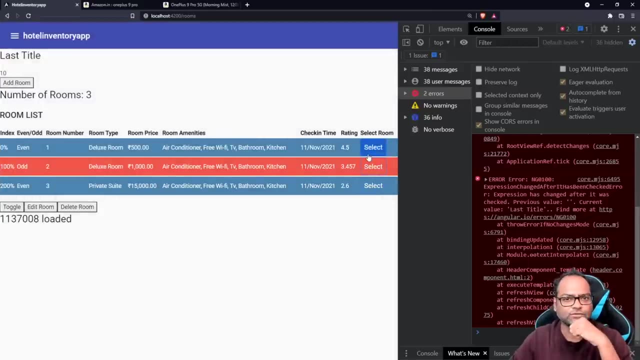 So. so let's go to the UI first and we'll go to rooms And remember, we added the select button. So what we'll do is, on click of the select button, we will redirect the user to uh another uh view where we can see the information about this particular page in uh, as we move forward, we will re uh, we'll actually change this button to book now. 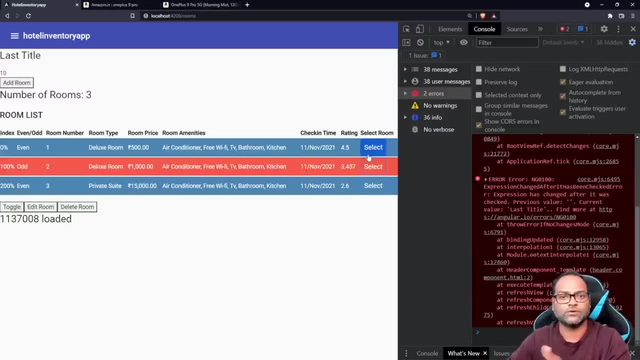 And uh, so users can not use this. but let's say it's a hotel inventory management. So the hotel, uh, receptionist or anyone can book the hotel from this particular button, So they know which particular room number is this and then they can just enter the information related to the user. 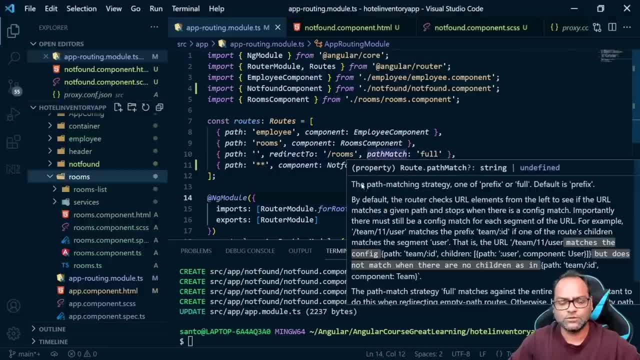 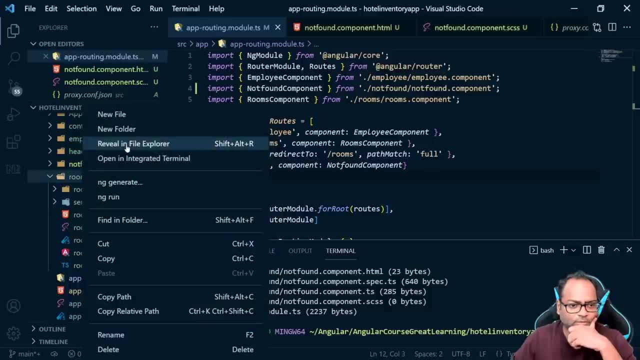 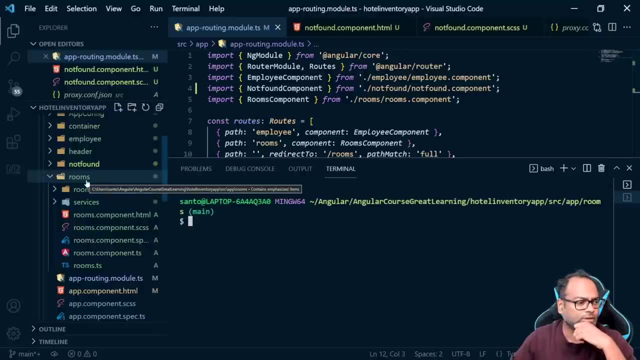 And that's it. I mean the guest, and that's it. So let's go back and what we will do is I'll create a new component here. So let's go to open and integrate terminal. Remember one thing: I mean I'm uh, I'm uh creating the components which are related inside the same folder. 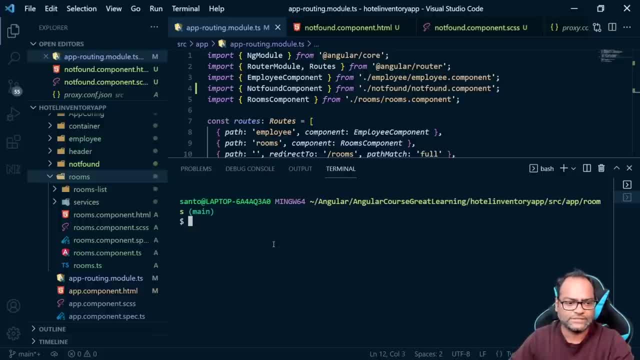 For example, right now I'm going to create a room booking folder, which is, of course, related to room. So I'm keeping this inside this folder, So I'll say this is NGC and I'll say this is rooms. Now we have this component available. 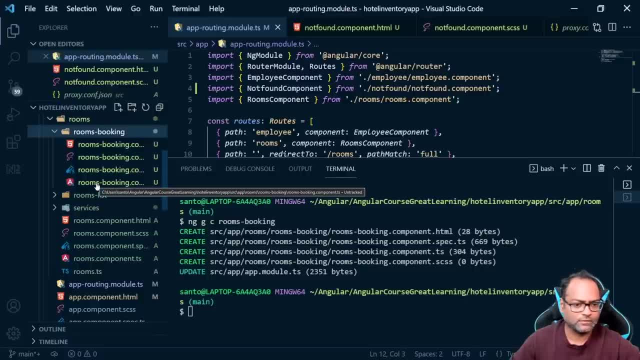 And So now we have this component available, Now what we have, Okay, What we have to do is we have to redirect, whenever we click on that, that particular select button on this component. So, but that particular ID will be, of course, it will be dynamic. 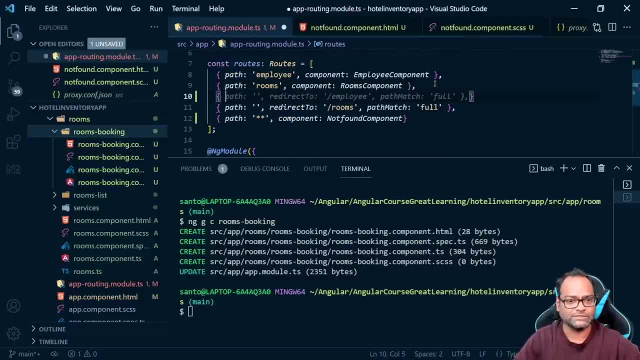 We don't know the ID by default, I mean in advance. So let's see how we can do this. So it's a path. rooms: Of course, rooms will remain same because that's the main URL at main endpoint slash and you can put colon ID. 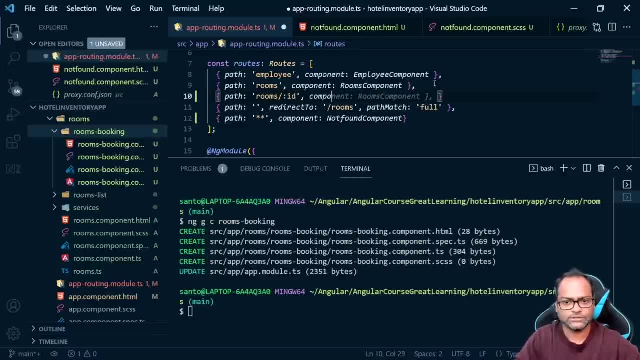 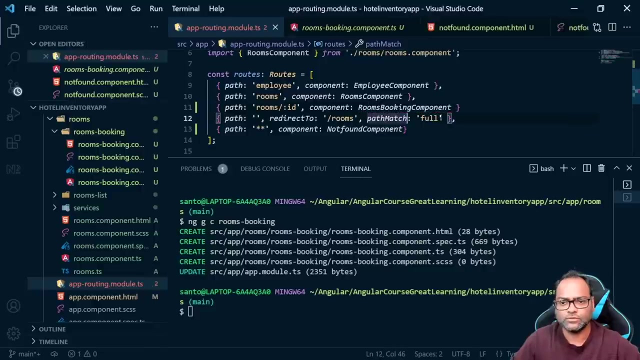 And let's see what the purpose of that particular component or colon ID is- smooth here. And then we'll say component and we'll say: this is rooms booking. Let's add this to module And this is this, So a room slash ID and then rooms booking component. 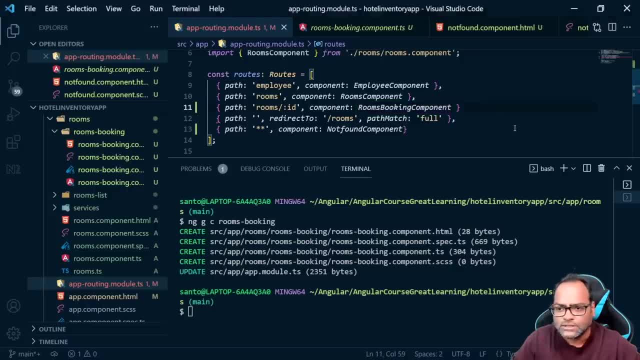 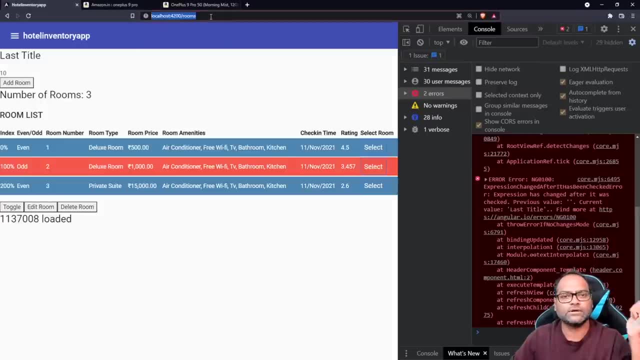 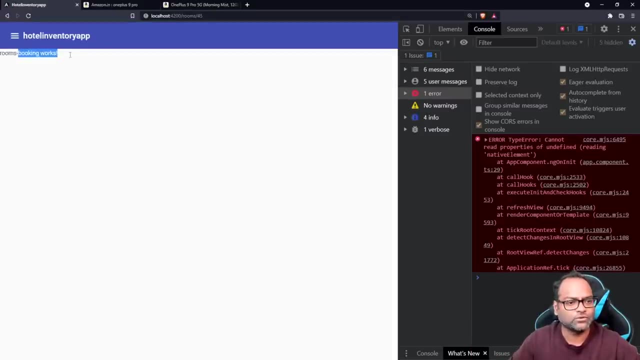 Let's Let's test this right now. And is there any missing thing? Yes, that's a comma missing here. Let's close this. And now let's try to test this first how we can test it. I can just enter whatever I want to after room slash and you can see it says rooms booking works. 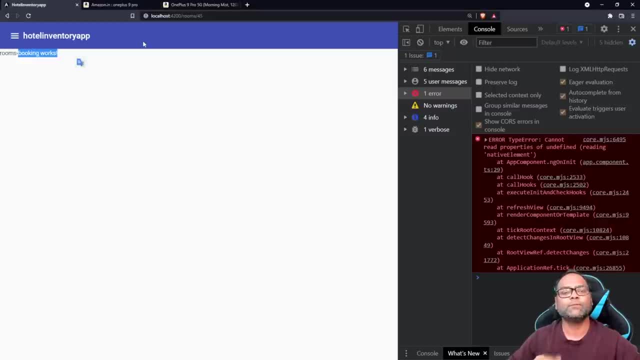 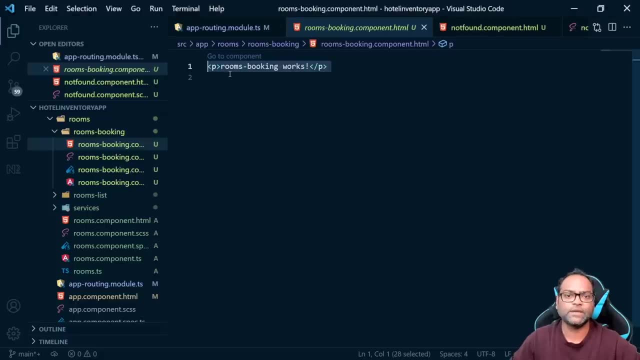 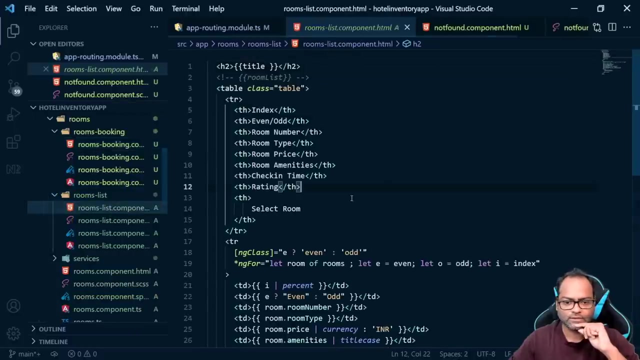 And from where it is coming. it is coming here, So it means my route is working fine. I mean I can enter whatever I want to after this and it will just redirect me to rooms. booking works Now what we have to do is we have to make a link from this rooms list, right? 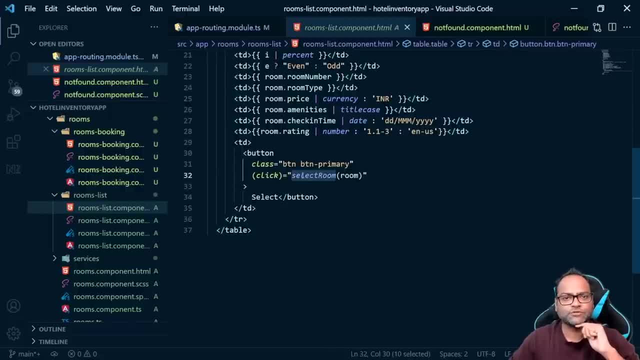 So whenever we click on this particular button select room, we should be redirected to that particular component. How we can do that, Let's see. So there are multiple ways. Uh, I can just use router link. Remember we, uh right now on select room, we used to actually send the data back to the component. 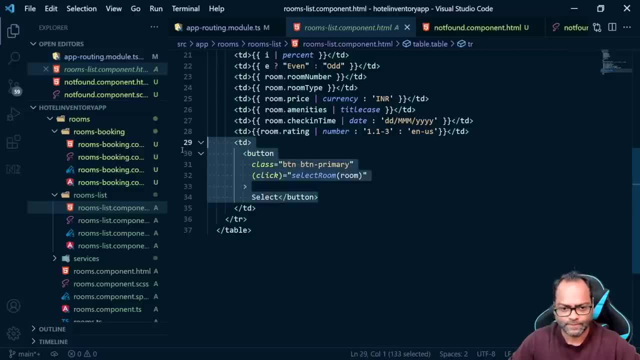 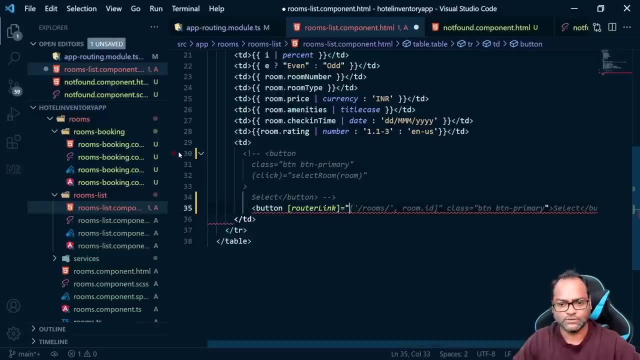 So what we will do is we'll just uh comment this out, Okay, Okay, And we'll use button now and with router link right now, uh, the router link value will be dynamic. So I'll put: a box is equals to, and then here I can say: rooms. 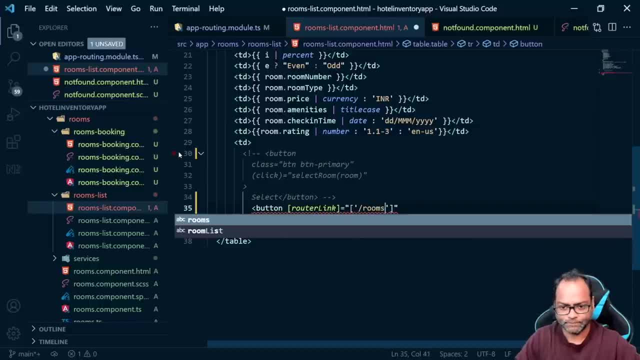 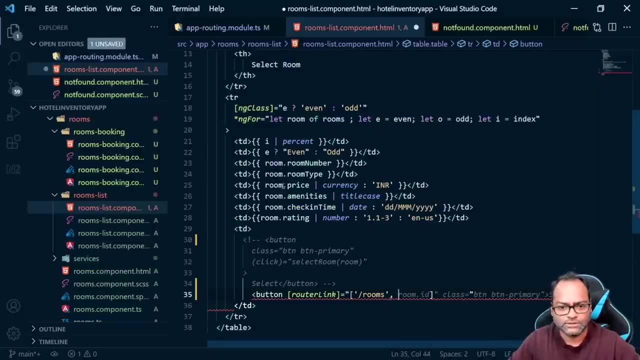 So I can say: slash uh rooms, And the next value is the ID which we want to pass. So we already have that particular ID, which is room dot ID, if you remember. So here Boom, And why We don't. 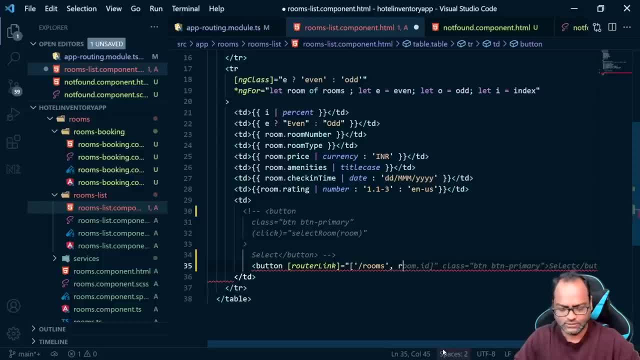 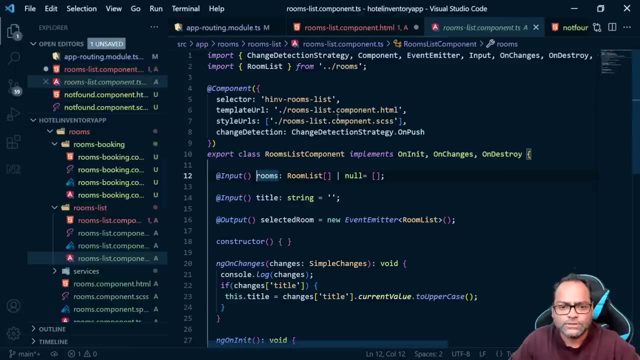 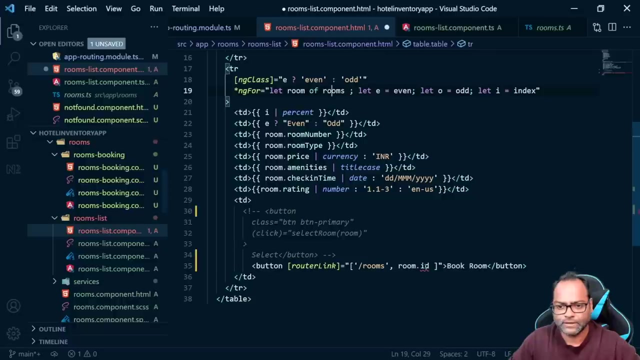 We don't have ID. Anyways, we will say room dot ID and let's close button and we'll say book room. Okay, Somehow it says rooms does not have ID as possible room number. Okay, Sorry, So we have a room number. 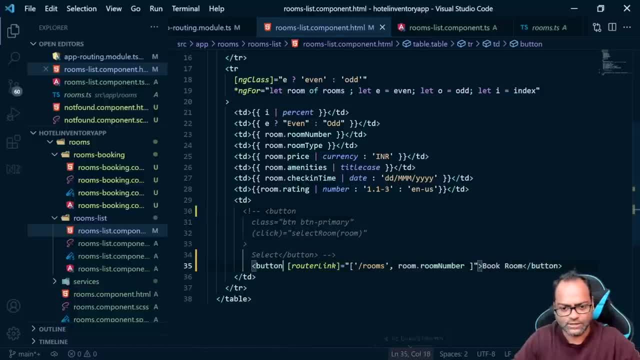 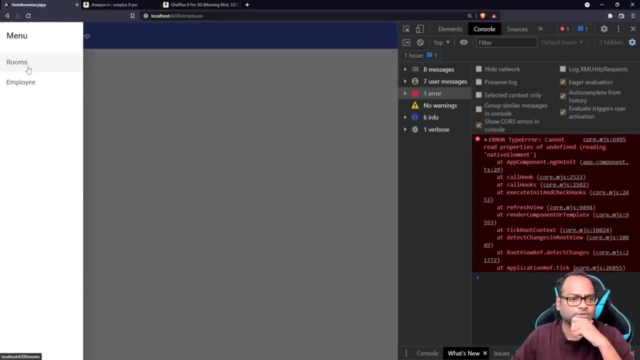 And I'll also add a class. So let's add the class. uh, BTN, BTN, primary. Let's use the same one. So let's go back to our employer. Sorry Rooms. Now we have this book room. I play button available here. 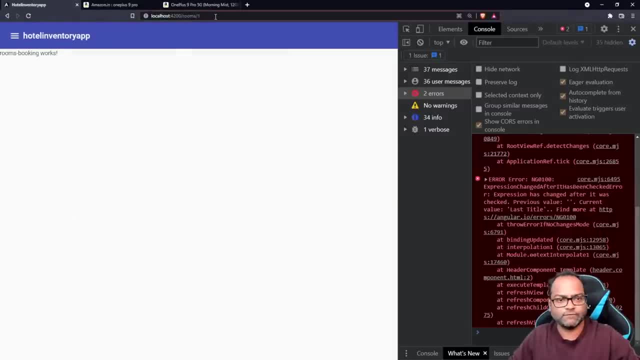 Let's click on one of them and you can see room slash one. So you have the values available here. So let's go back again and click on rooms book And we have the ID as two available here. So now we have configured a dynamic route. 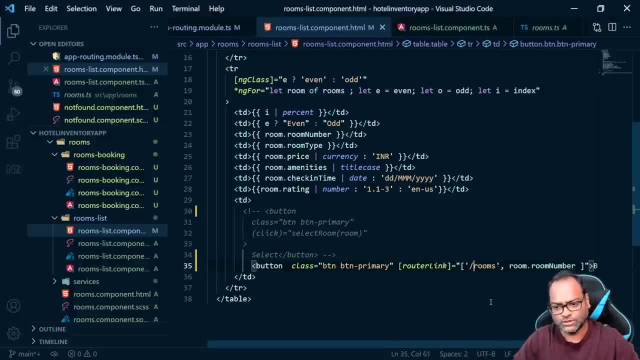 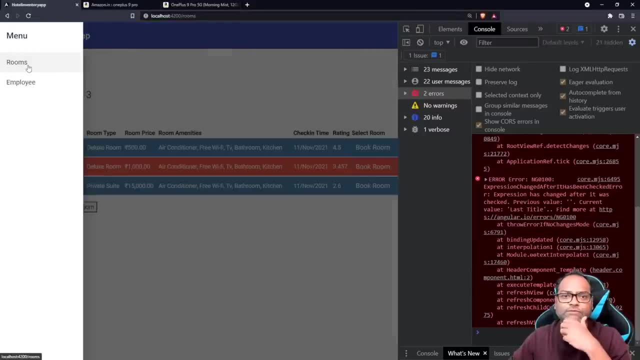 Now we can actually navigate between that. but let me show you one more thing. I'm removing the slash here and it has a purpose, So let me show you, because this is something which you may face in your real-time application. So you can see now what, what is happening here. 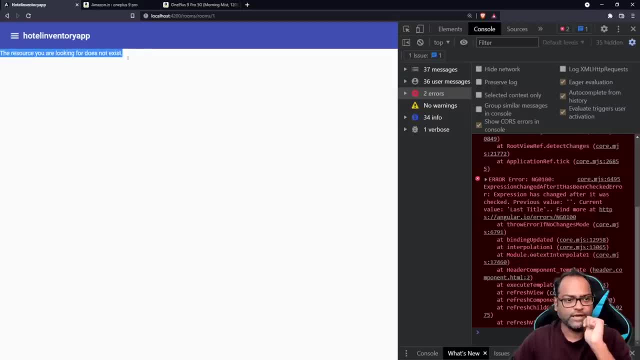 Now I'm not redirected to rooms booking page. Remember, I'm redirected to 404.. The resource you are looking for does not exist. Why? Let's say, let's see the URL found the issue: Yes, rooms is twice Why so? why it was working before. 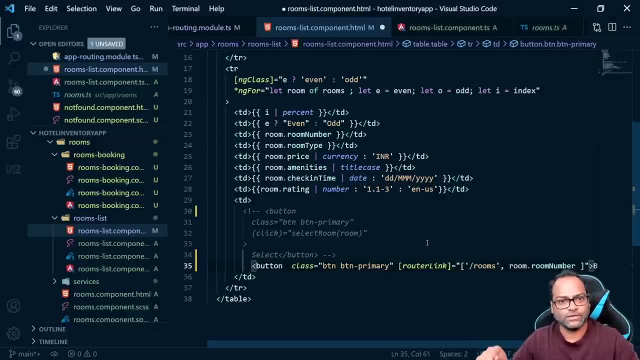 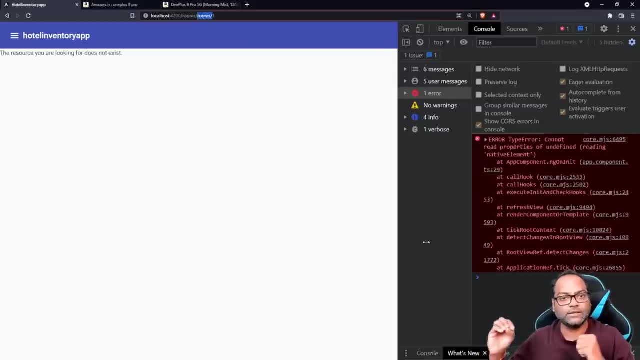 So whenever you say slash, it means the route should start from here by default. the uh routing functionality works in a way that it will always append the previous URL, which is already- or sorry, previous uh. you can say: uh, the parameters. there are parameters which is already available. 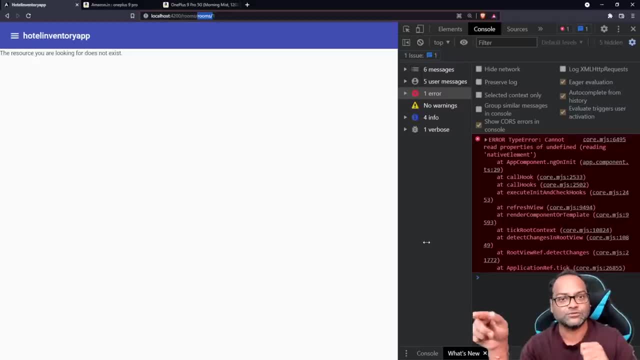 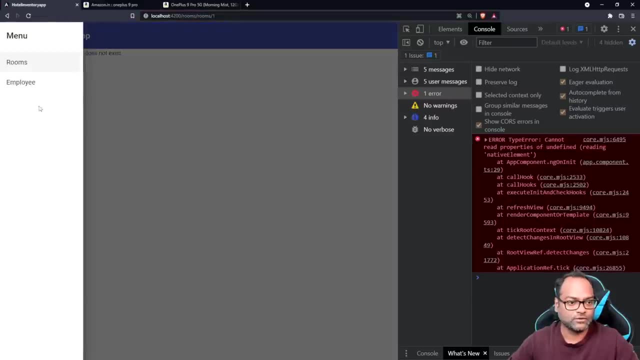 That's the reason it was like so doing room slash rooms because, um, we said we we don't have slash right? So it will say, okay, the earlier parameter is rooms here, right? So it is it is. it has a rooms. 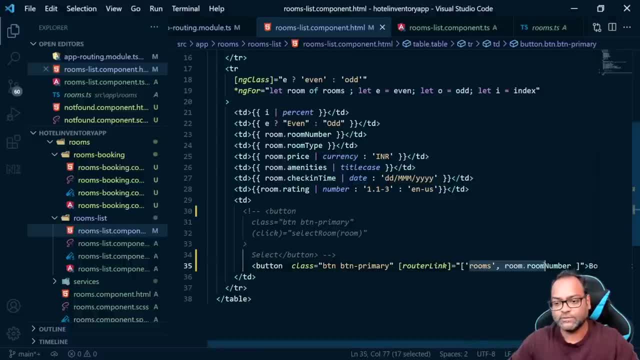 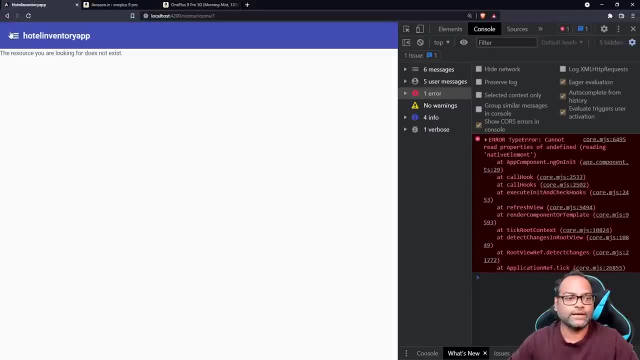 If I click on this, it is saying just go ahead and add these two parameters to the URL. When we put slash, it is saying just start from here. So, whatever the URL is, I want to redirect to rooms slash ID. 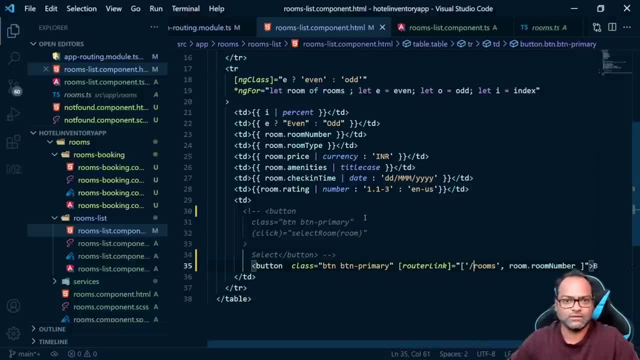 So this is the difference. Remember, uh, really, uh, keep this in your mind or you can just revisit the video again in case you get this error, uh, in future. So, uh, we have configured dynamic uh URL. 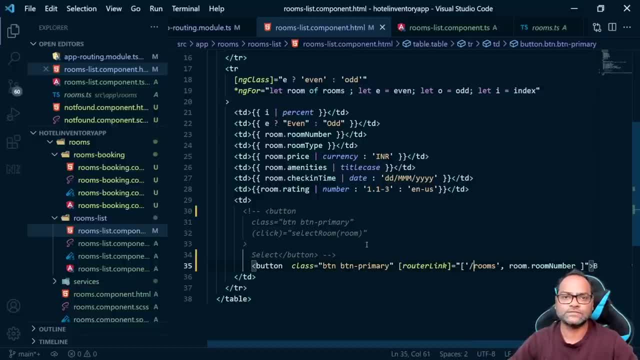 We are now able to redirect to- uh, the component as well. What next? What next? What do you think? What should be the next step for us? Yes, you guessed it right, You. we need to get the ID right. 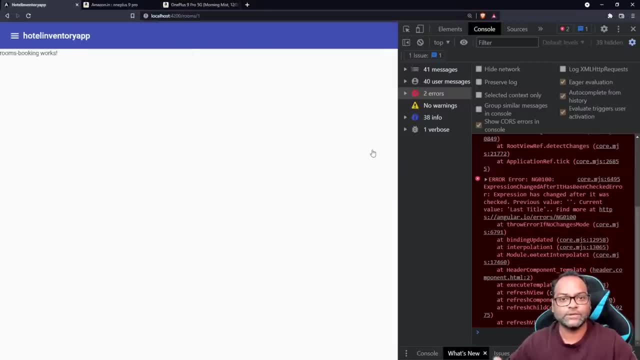 So, whatever ID we are passing, in case you want to book this particular room, we need this ID. We need to read The one or two, whatever value is available into the parameter. So let's see how we can do that for that. 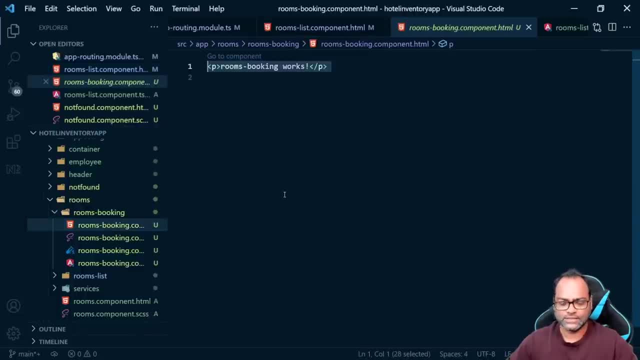 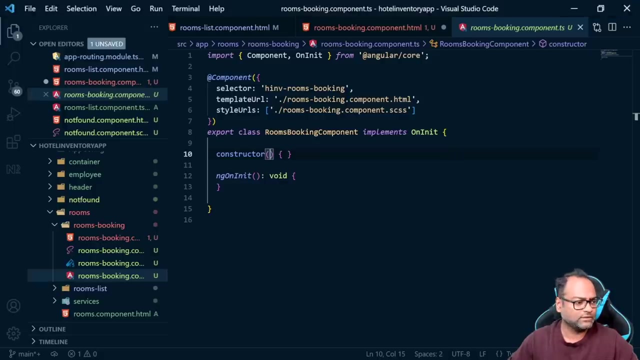 We'll go back to rooms component and let's say, uh, what we'll do here is we'll put the ID. Uh, I'll just do ID right now and let's see how, how we'll read this ID. I'll go back to the slides and 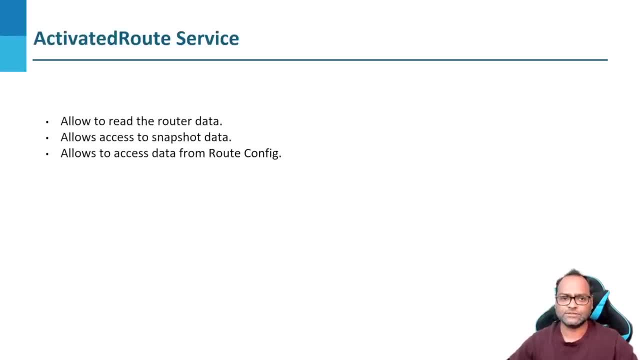 We'll talk about a service called activated route service, because this is what we are going to use. Remember so what activated route activated route service does? So it allows you to read the router data, whatever router data which is available inside your application. 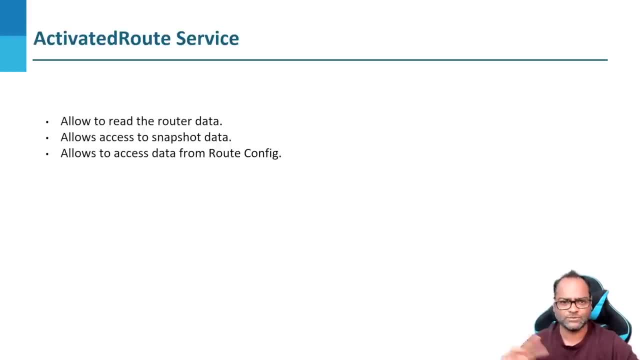 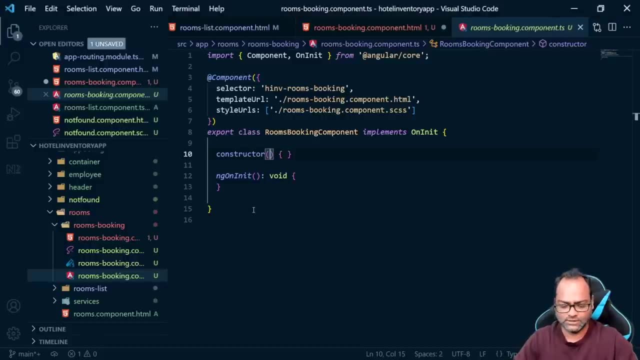 You can also access the snapshot data. So we'll talk about what snapshot and the other data is, And then you can also access data from route config. We will see all these examples, but let's do first what you want to do is: we want a, we have. 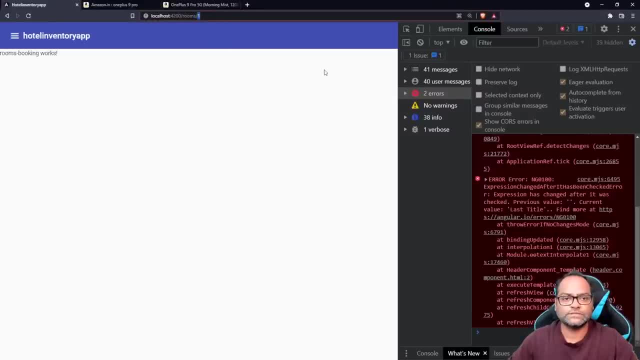 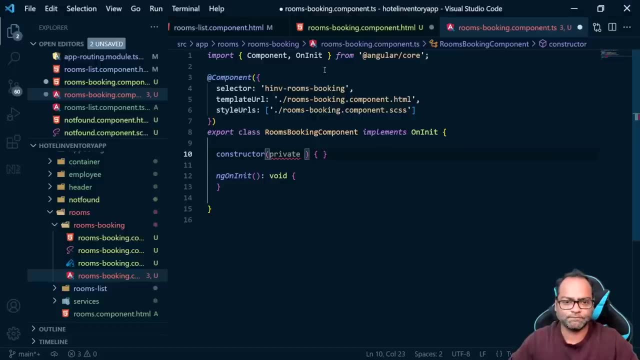 Right now, the value, which is which we are talking about, is it is available inside our route, right? So we want to read this one, So I'll say private. this is a service and it is available by default by, and provided by, angular router. 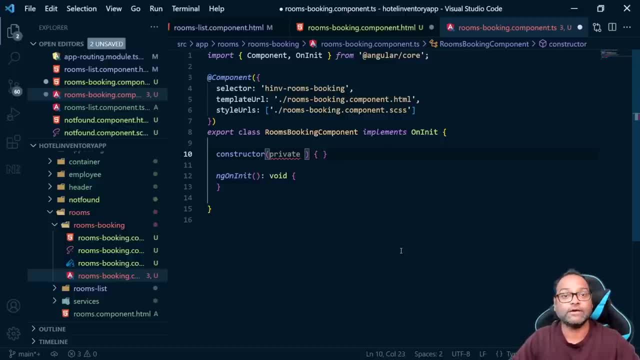 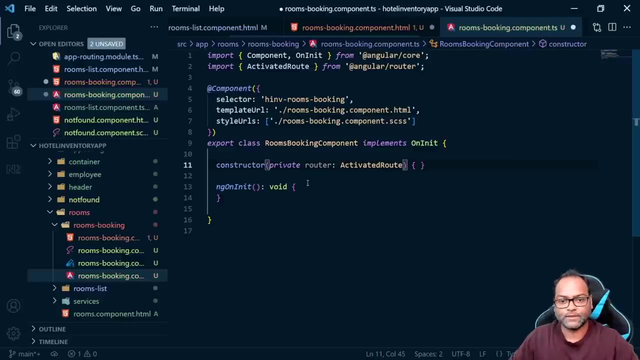 So you don't have to do anything else, You we have already. we have already imported the router module, so we don't need to register anything extra. So I'll say this: uh uh, router Which is activated, route right. 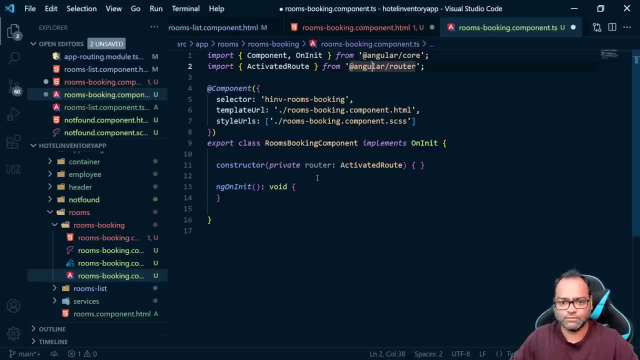 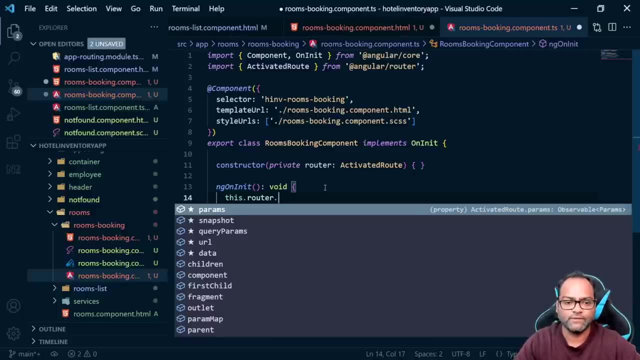 So we have injected the service and this should come from angular slash router. Remember this. And now, uh, here we'll say this: dot, router, dot. So there are multiple parameters which we have And the ones we are. the one which we need is we need tabs and then in parents, see this: 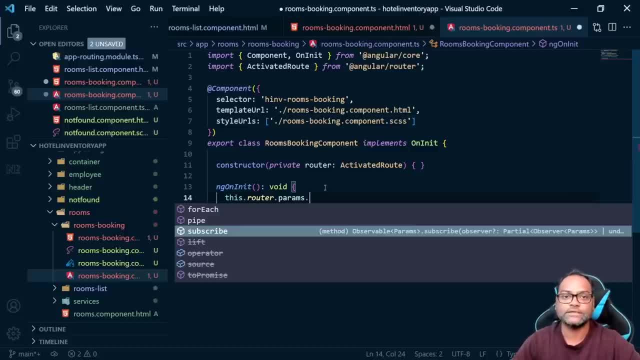 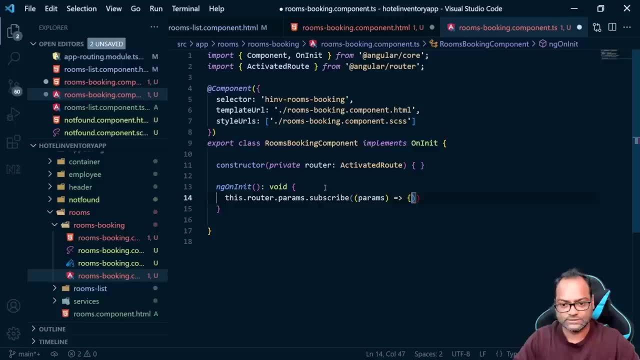 So it's also an observable. Yes, So router data is an observable, so we can say subscribe and let's See. uh, I'll say uh, let's say parents and see if there's an extra closing. Yes, And console dot log parents right now. 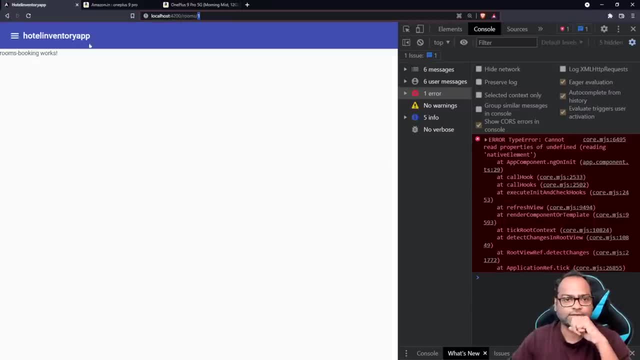 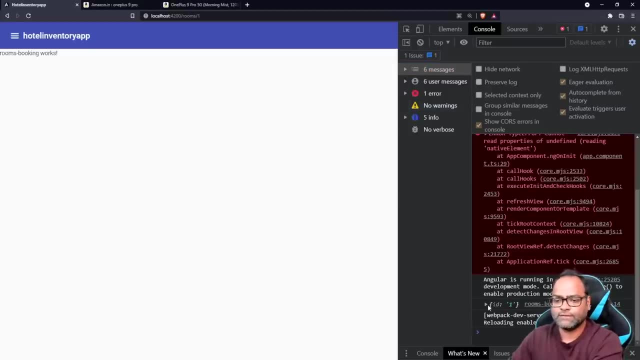 We'll just do this. Let's see what we get here. So console and we have this right, So we, uh, let's submit. so we have ID and one, so it gives you key value, but from where This? 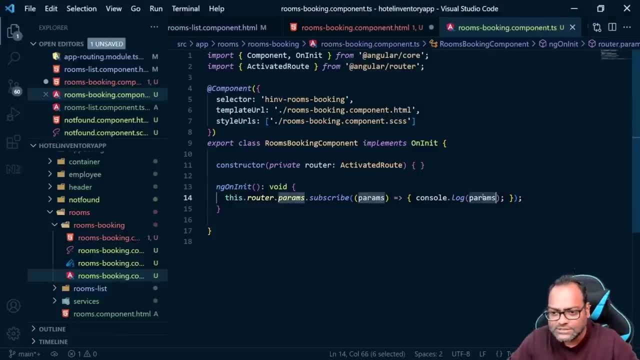 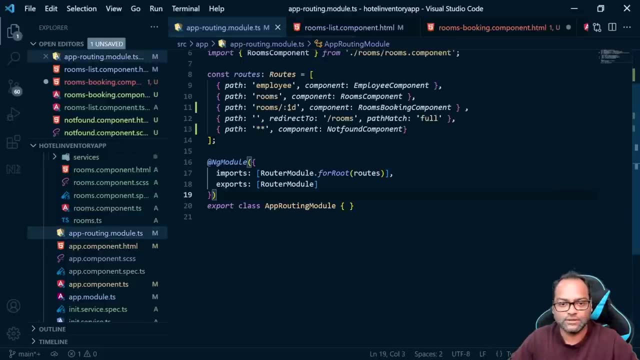 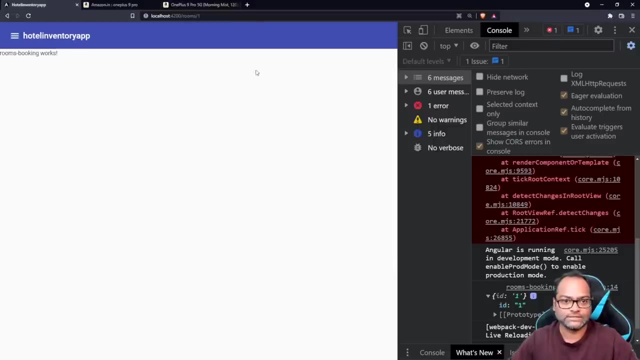 This particular ID is coming from right. We are not seeing this. uh, just record and read ID. Let's go back to our code base and let's go to the configuration. This is the ID. So angular, remember, knows that. okay, this particular key, whatever I'm passing here- is actually defined as ID. 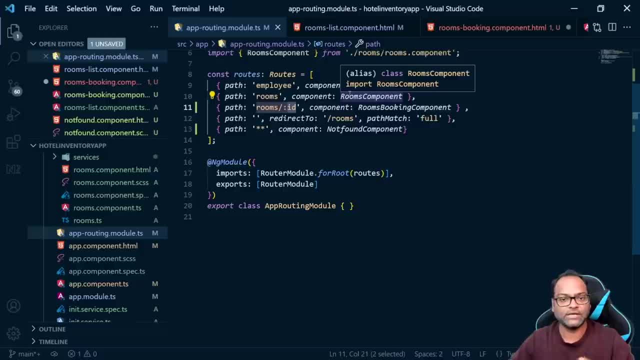 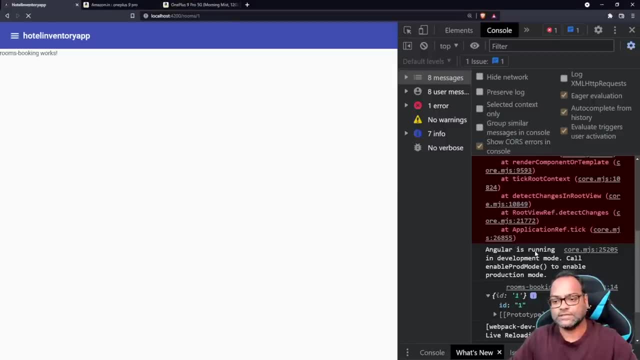 You can name it whatever you want. It doesn't need to be ID. I mean you can just say room ID, Let's try that Right. So we can say, uh, room ID, And let's see here. So you will get it as room ID, not ID. 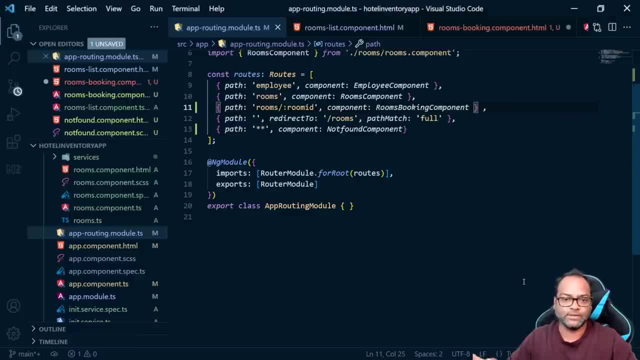 So keep it whatever you want to should be. I mean, um, it should describe itself right. I mean, here we are talking about room, So it doesn't make sense. I mean, even room slash ID does make sense, but just not to get confused. 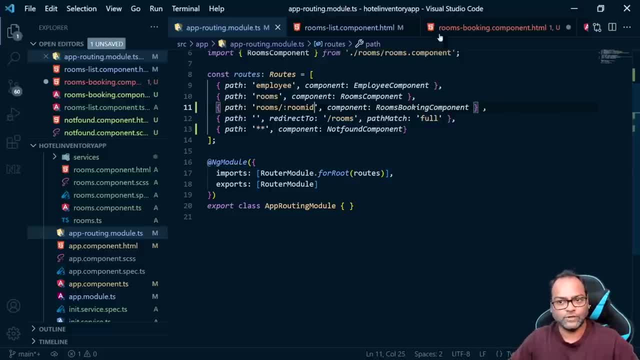 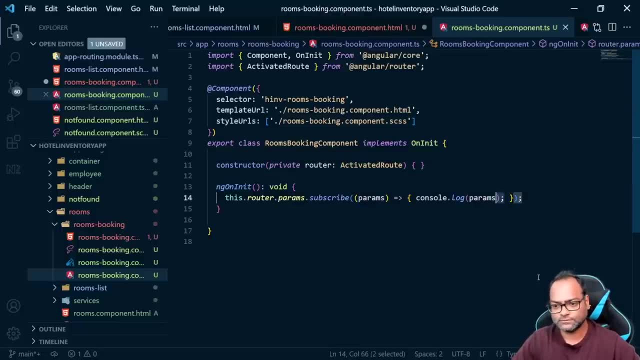 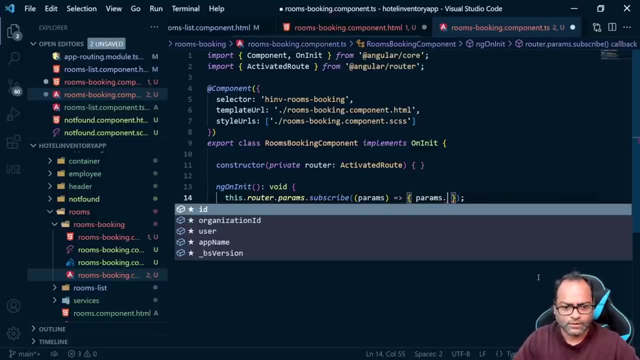 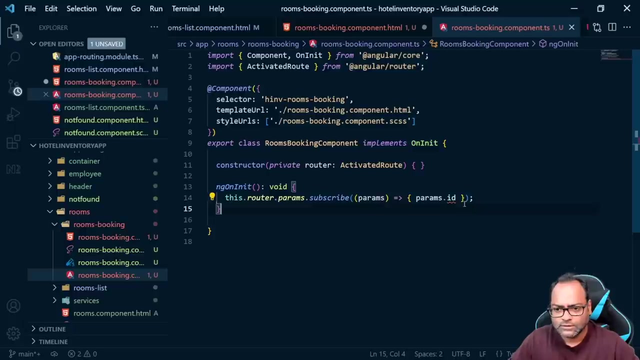 You can just keep it whatever you like. Now we, uh, now we know the key. Now let's try to retrieve the values. how to get it? So here you can say: parents, Dot, get Okay. There are multiple ways. 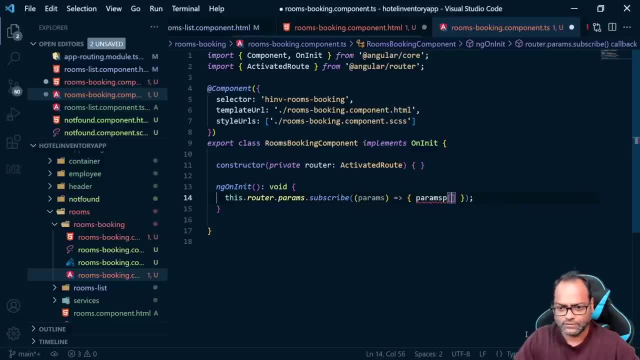 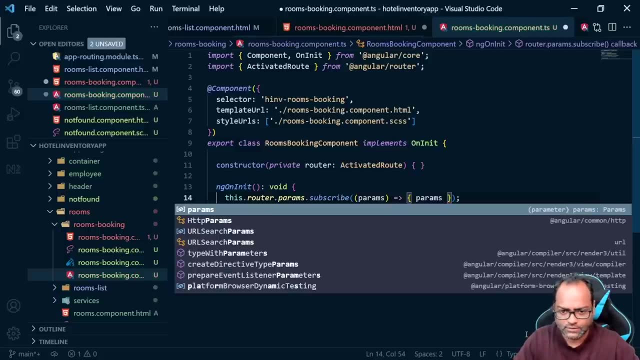 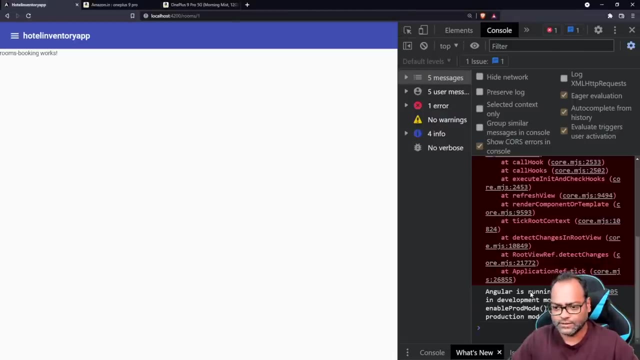 So we can do this one. Let's try it with um parents Dot. No, this is not the one. Okay, So parents of room ID, and let's see we need to, of course, do a console dot log. 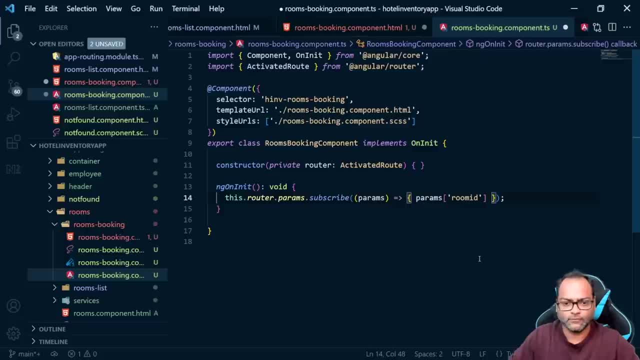 So let's try, let's do one thing. So I'll say, uh, remember, we already said, uh, we'll be using a variable called ID and this is number. So I'll say this dot ID is equals to: Okay. 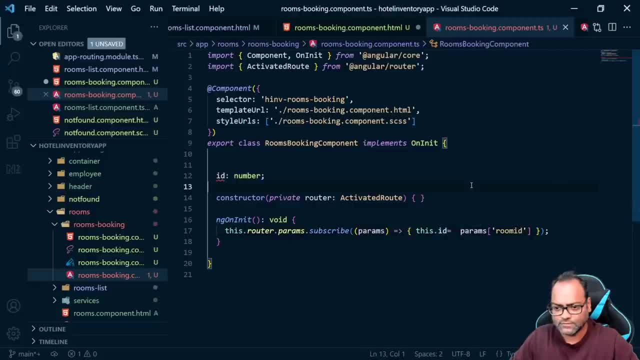 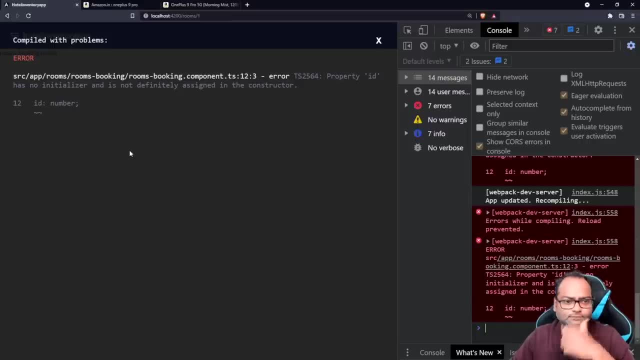 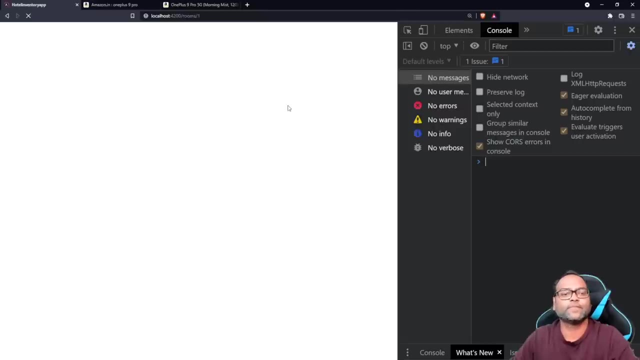 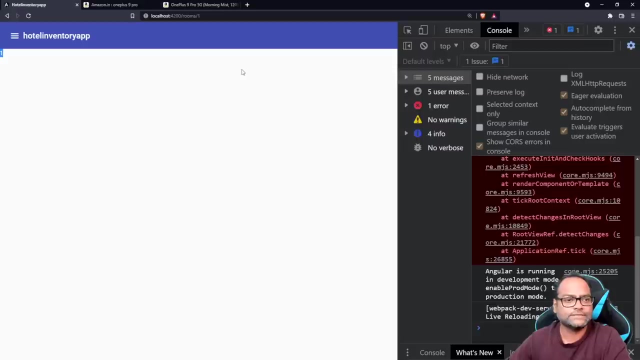 Parent of room ID. So let's see, and we will save this as well, The template one: Okay, It has no initializer, So and say: this is default to zero and you have one available here. So you can see, uh, the value which is available inside our route, uh is now we are able to capture. it. 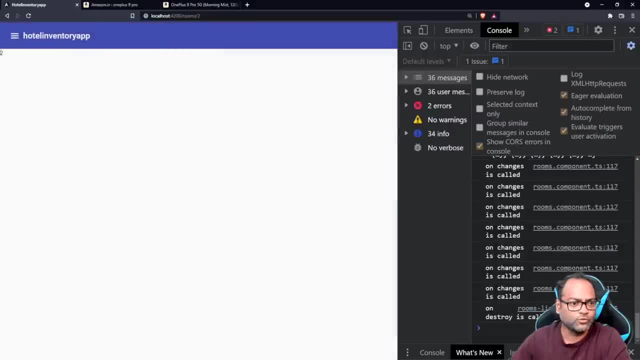 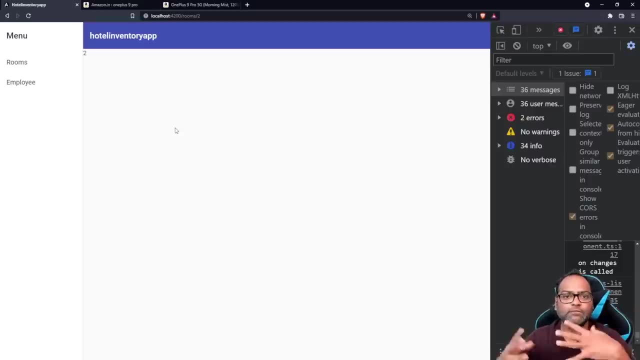 So let's go back, click on rooms, click on room Do, and the value two is available here. So this is how you can actually uh, go ahead and access whatever dynamic parameter you define inside your word. But let me show you one more thing here. 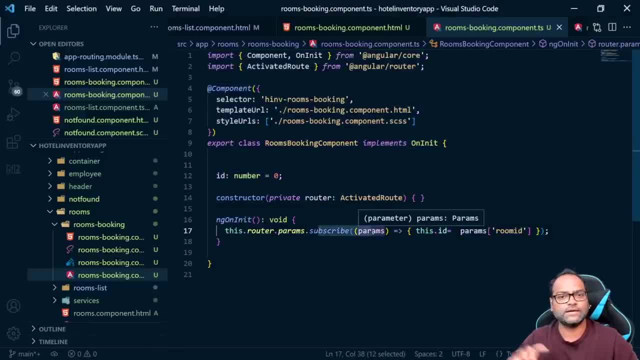 So here, uh you, uh. remember we always uh. we said, while talking about RxJS, you should not subscribe. Remember uh by talking about uh observables. we said we should not subscribe. It will lead to memory leakage. 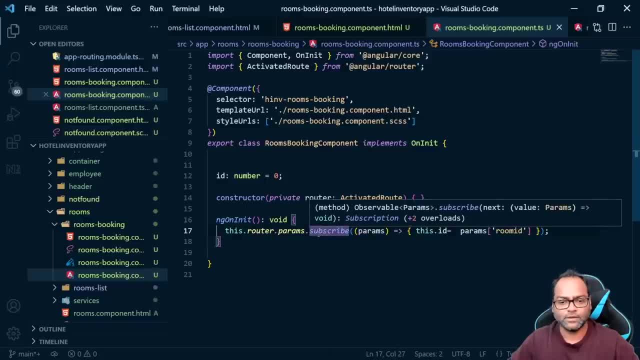 So how we can actually Make sure that, uh, uh, I mean how we can avoid this particular subscription. So there are ways, of course. the way is using the RxJS operators. So here, what we can do is we can actually do something like this: 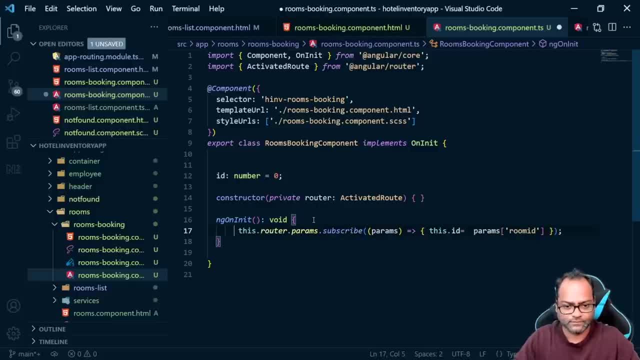 So I can say: um, this dot ID is equals to, I'll say this: dot, uh, router, dot. Let me show you snapshot as well. Sorry, We actually wanted to discuss about this as well. So params, snapshot dot. params of room ID. 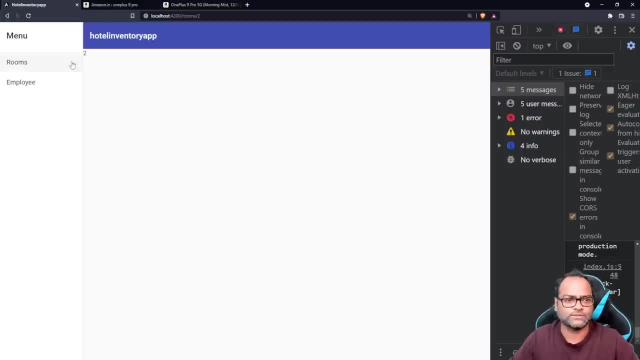 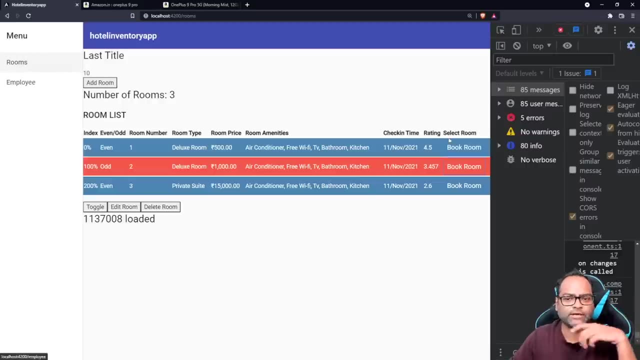 And let's see snapshots and then we'll come back to the subscription. So let's go to rooms and click on one. Let's go back to rooms and click on two. So you might be wondering: okay, if I'm able to get the data using snapshot, why should I go ahead and use subscription? 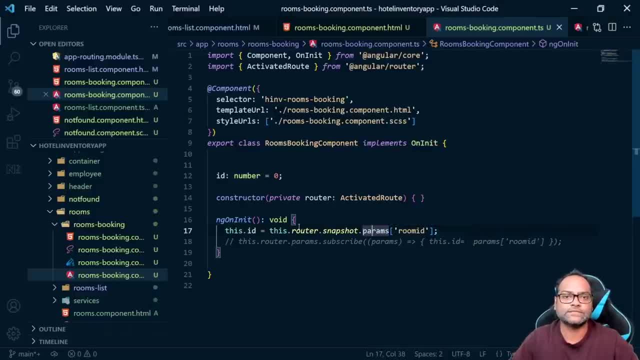 So remember, snapshots will never update The data in case you are changing the value being in the same view. So whenever a new value is submitted by anyone, that value will never be captured. right now We are actually migrate a, we are navigating to another view. 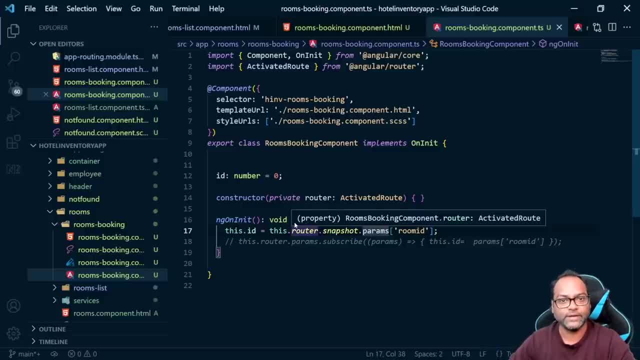 So it is. it knows. okay, we are coming from another view and I need to update our. take this data from snapshot, So this will never receive a new value, in case it is already in the view. Remember this because in case, uh, in future we will talk about child components. 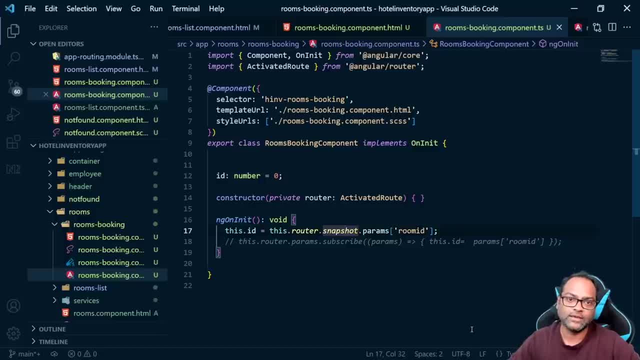 And if you try to access using snapshot, you may uh, get into issues right Where the value will never be updated. So this is snapshot, but this is not what we are looking at, So I'll set this dot ID. 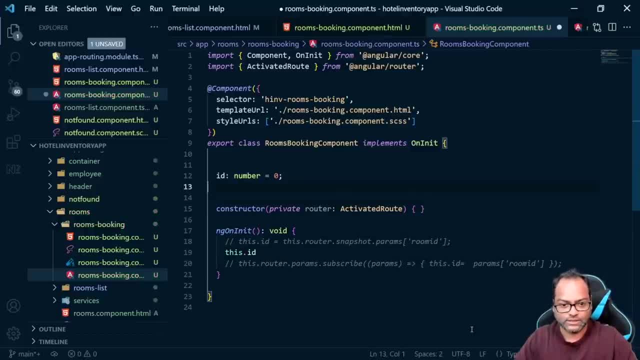 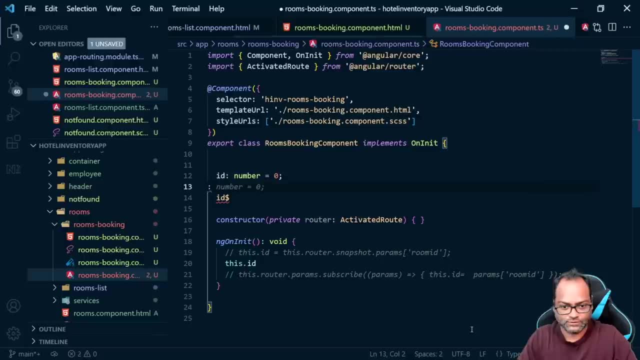 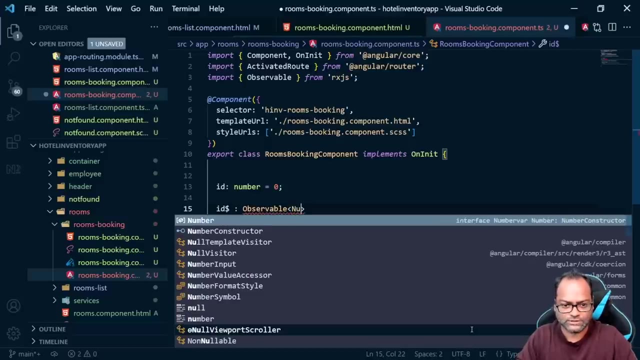 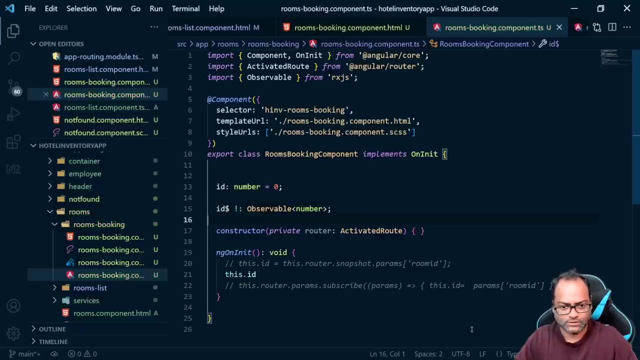 I'll create one. uh, yeah, let's create ID. stream is equals to uh, which is type of sorry, type of observable, of number, because we know what this is going to be. Okay, It's going to be number, and we put this here and let's see. 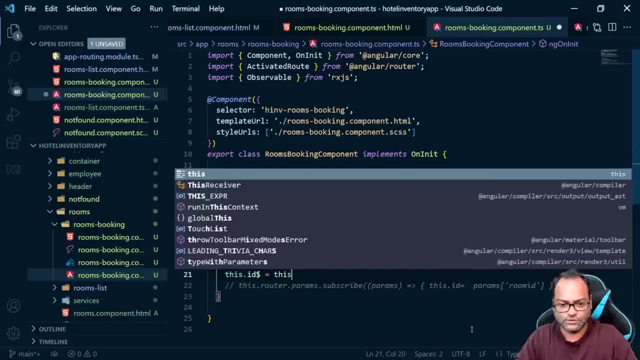 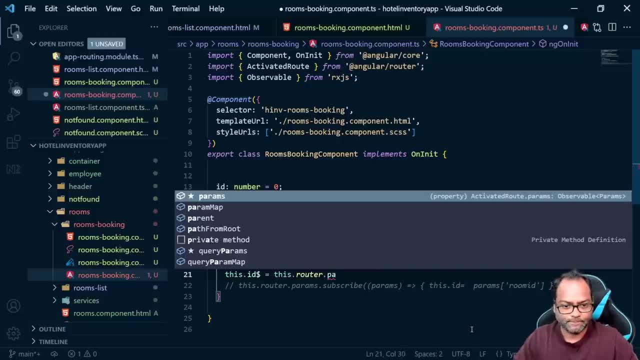 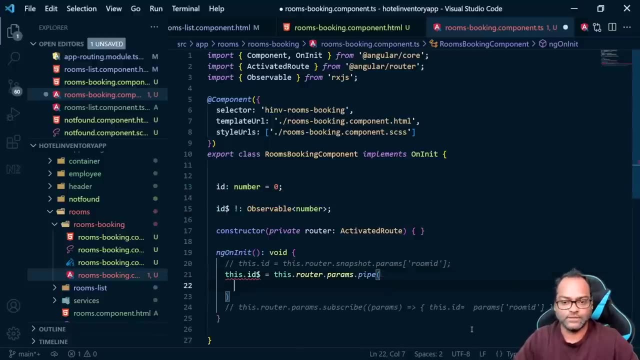 So you'll say: this dot ID, which is stream, is equals to this dot router, dot. parents thought: Now we'll use pipe because we don't want to subscribe, and here we will use something known as there are multiple operators we can use, We can. 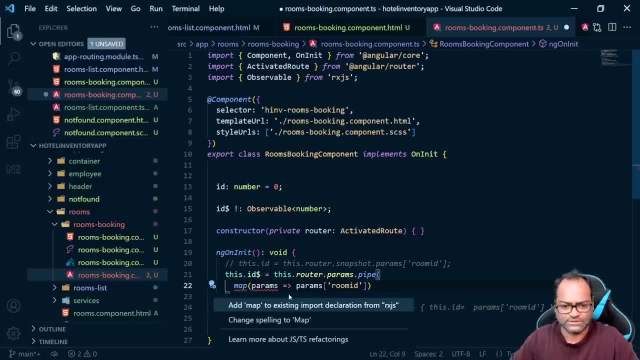 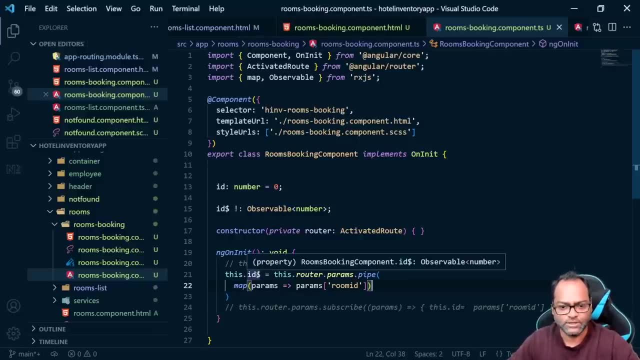 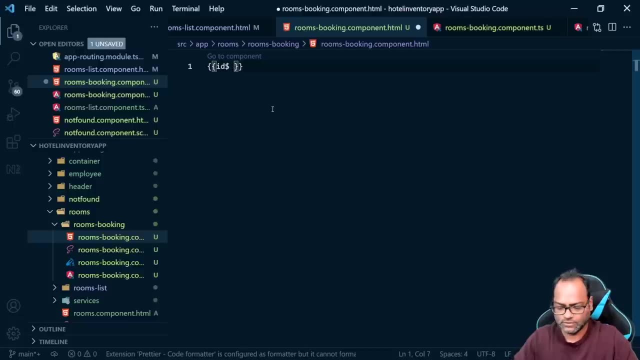 We can just use map, right? So let's try, let's go with map. I mean, this is the, this is the easiest one, right? So we can say map and you can see the ID. Uh, it says it will be type of number because it knows the type. and let's move and use this ID by a sync, right? 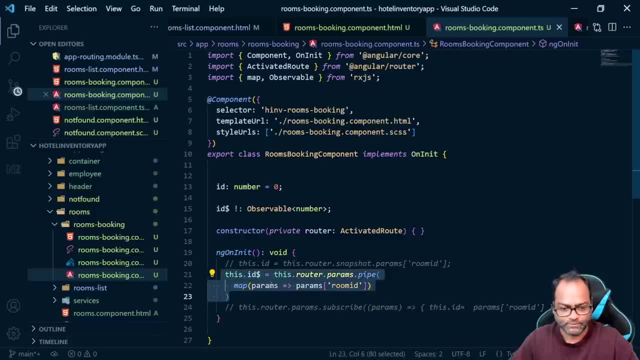 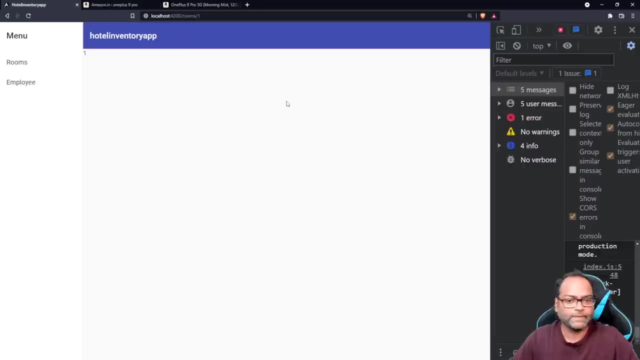 So what we have done here. so we said now we are not going to subscribe manually, We can just do this. Let's, let's try to avoid this and let's do this. ID is equals to this and I'll come in this one format and, uh, let's see the application. 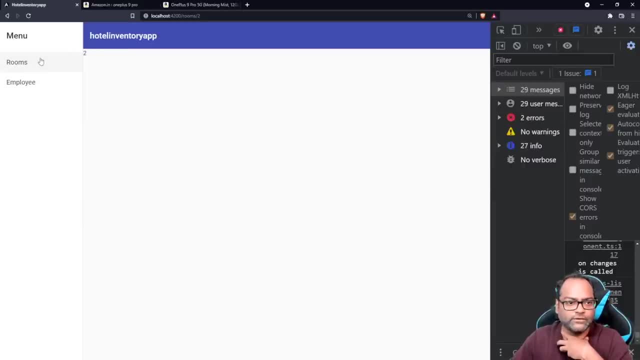 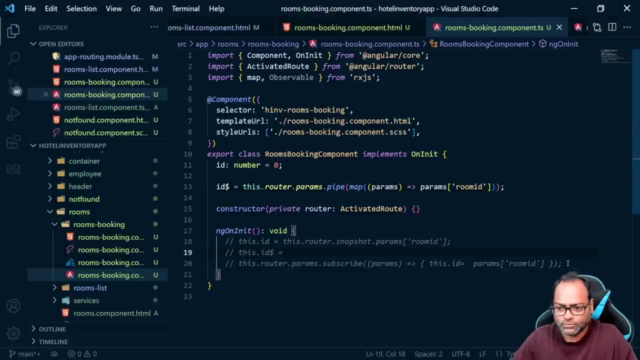 So you have the value when available here. click on rooms and values to click on here and values three. So we are still able to get the value, the parent value, by using a sync pipe. We are not, We, Uh, we are not subscribing anymore and uh, we also saw how we can get the data from parents using the activated out service and what else. what else here? 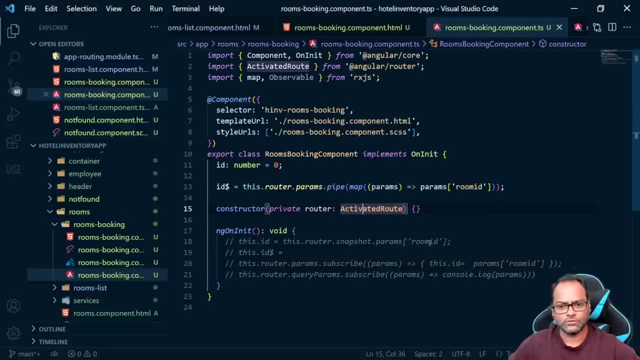 Uh, let's talk about so here. let's talk about one more thing. So right now we are using this parents property, right? But there is one problem with parents property. What in case? we have multiple values available as part of your query, your parameters, right? 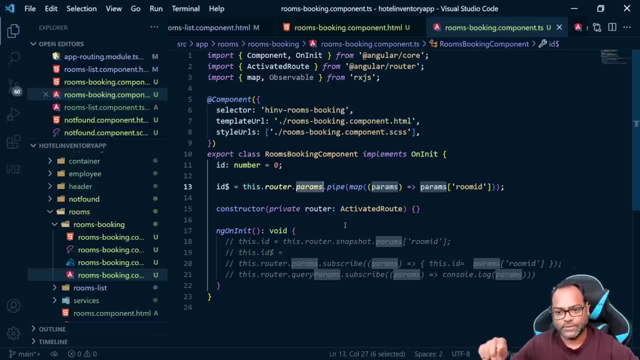 What, in that case? what you will do? of course, you can say parents of another value, but there is another uh API which is also available, which is more preferred than this parents. So let's try to use that particular parameter, uh or particular properties. 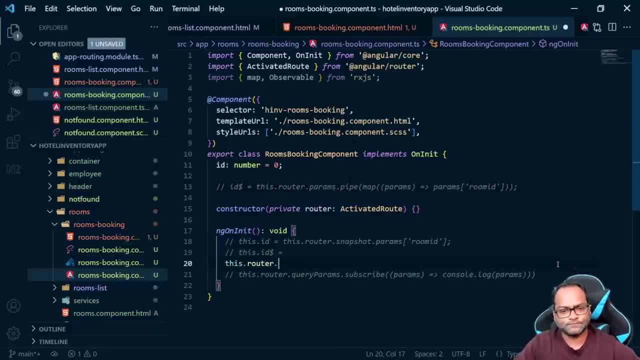 I just comment on, comment this, and rather than parents, we will use something known as parent map. Same, It also emits the opposite. It also emits the opposite. But let's see what is the different. what, uh, sorry, what is the difference here? 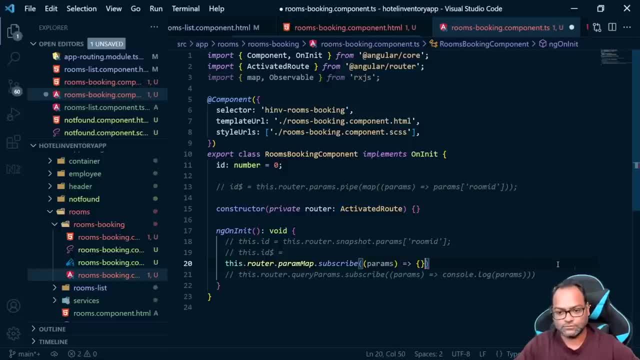 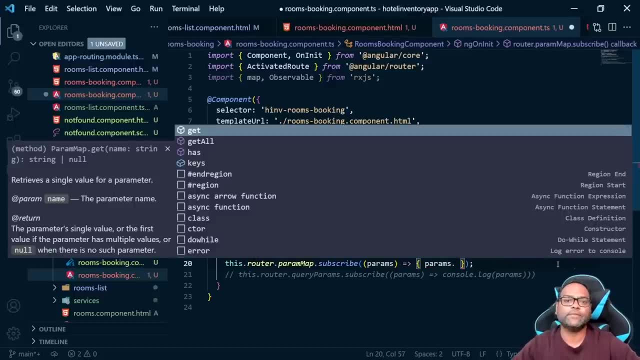 So it is a parents and to get the value here you can use parents dot. And now let's see this. So it has some methods like get get all has keys So you can, before even accessing the values- sorry, before even accessing the values- you can see if this particular particular key exists or not. 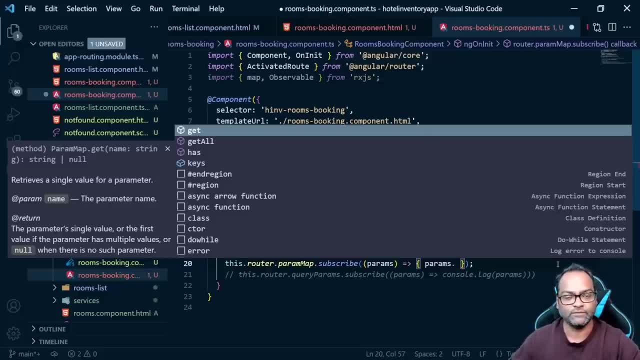 Right. It is really useful in case you want to retry multiple Information, and other information is probably, let's say, optional right. So you can just check if this particular key exists by using ash- sorry it has- and then you can access the value. 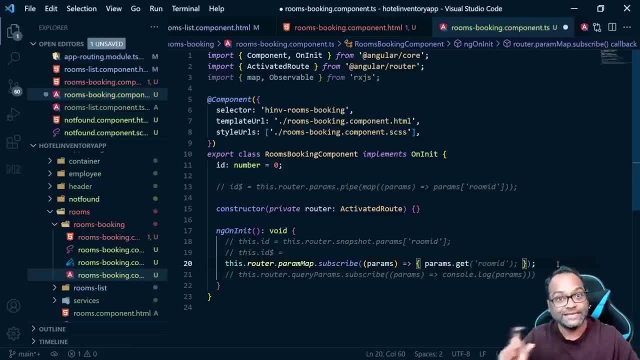 So here you can say get, and then you, you have to provide the key again, the key will be room ID. So this is how you will be writing it. But as we already have this code, what we will do is we will replace this using this one. 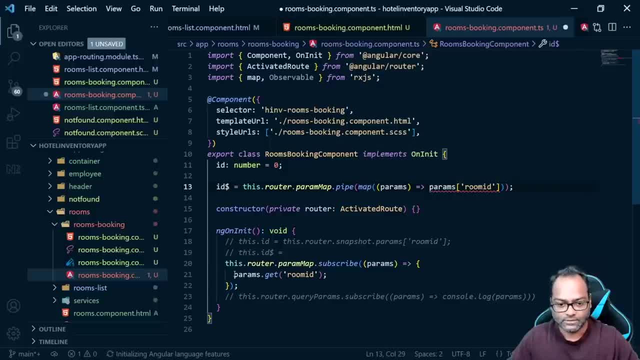 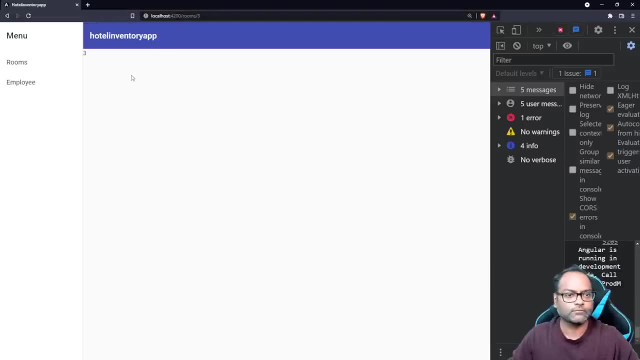 So you can say parent map and uh here, Okay, I'll say parents dot get room ID. and let's uh comment this out. We don't need it anymore, We just wanted it for reference. and let's go back to our UI. and we still have this working code available. 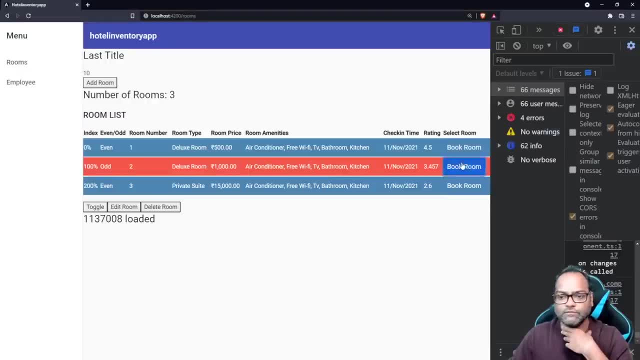 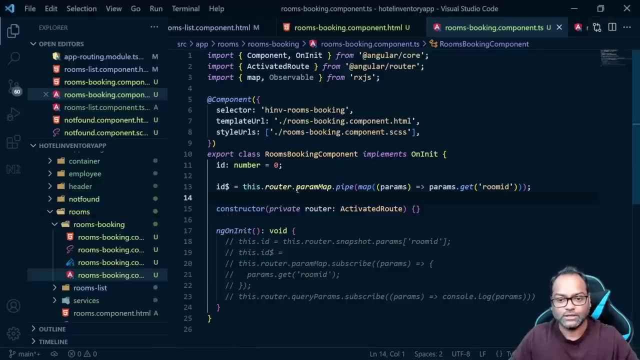 So you can see, uh, the values. whatever value we change, we are getting that value available here. So this is a preferred pattern map, because it does like more clean UI, rather than actually, uh, just getting the value like this, which may throw an exception in case the key does not exist here. 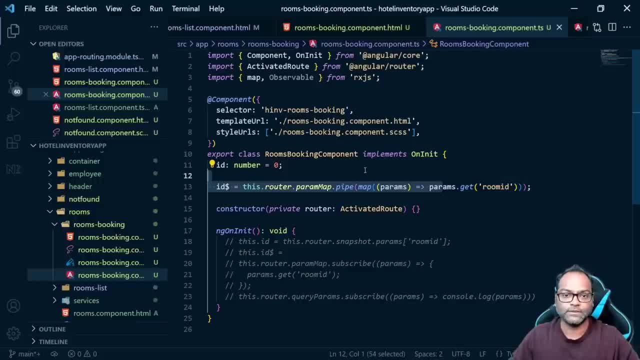 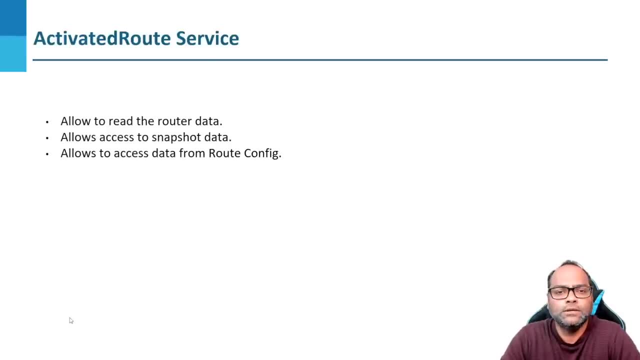 You can actually go ahead and check if this key exists and get the value. So this is from the dynamic routes and let's move ahead. Before we go ahead and utilize more services related to routing or more functionality related to routing, we are going to have some more views. 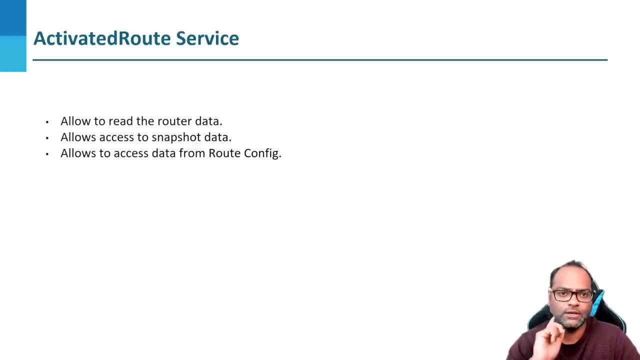 And for that, what we are going to do, What we are going to do is we are going to jump right now into forms. So what we will do is we'll create some views, uh, using forms, and we will combine both together. 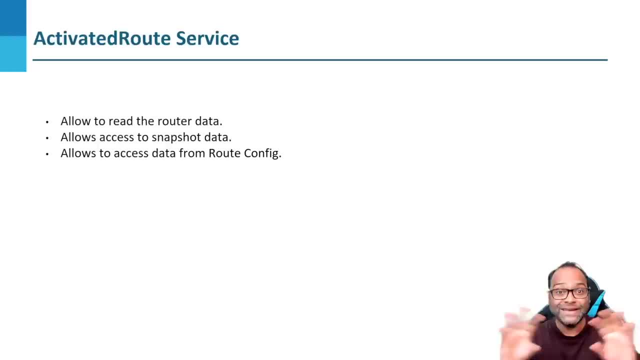 I mean forms plus routing, So we get a complete picture how our application looks like. So we are going to start with template driven forms. So let me uh, tell, uh, let me tell you this: first, angular has two types of forms: template driven forms, and it also has reactive forms. for me personally, I prefer reactive forms, but it's not like they- uh, one is one is bad. 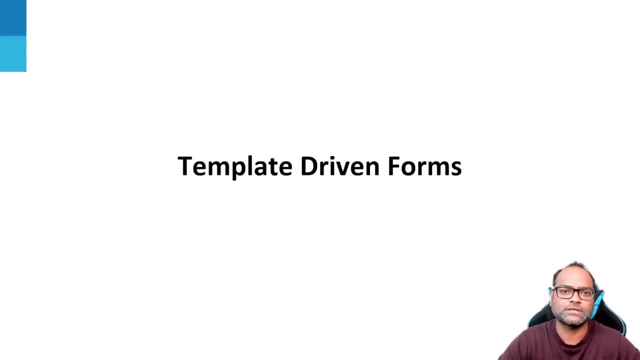 One is good. It's not like that They both are powerful. It's just on, based on your use case, what you prefer, or based on what flavor you prefer, right, So we will go through Both. We will create forms using template driven forms as well as reactive forms. 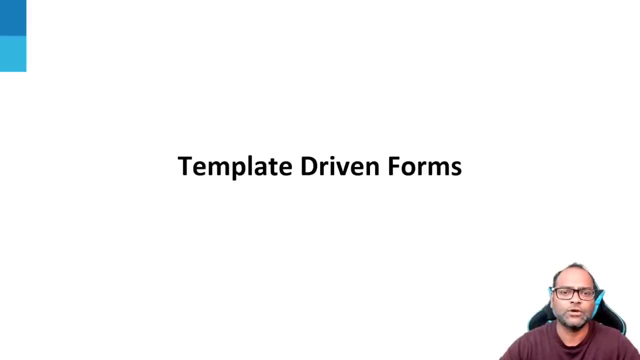 And, uh, you can choose by working on your application, which suits your team, which suits your application. So let's start with template driven forms first. So what the agenda is? we will set up template driven forms, We will see how we can add validation. 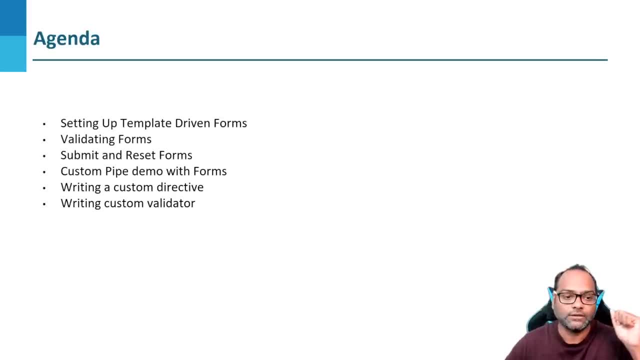 We'll see how we can submit and reset forms. We will uh see some examples. If you remember, we uh we saw pipes and we saw directives. So here we will see uh how we can use custom uh for how we can write a custom pipe, how we can write a custom validator uh and how we can also write a custom directive. 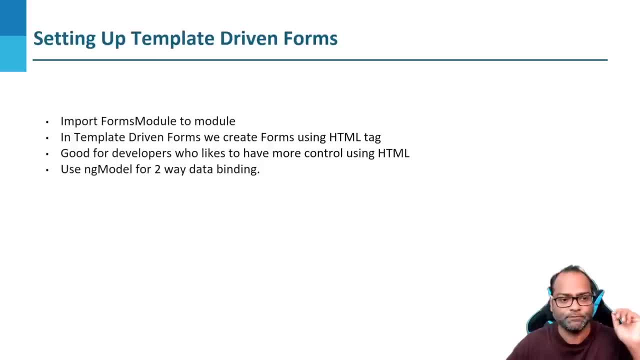 So validator part: it's related to forms, how we can validate forms. So let's see, uh and uh, let's go ahead and see how we can actually set up a template driven form and how we can create our first template driven form. 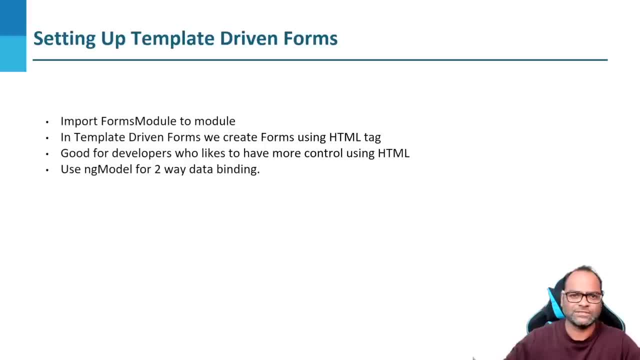 But what we will create. So, remember, we performed some crude operation- crud operation right- And we took an example of adding a room. So let's do that. Let's create a template, Let's create a template driven form for adding a room. 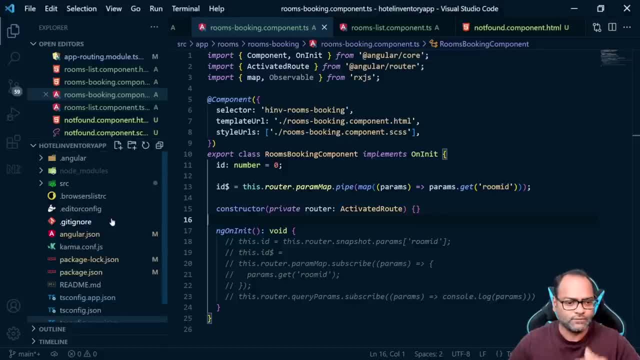 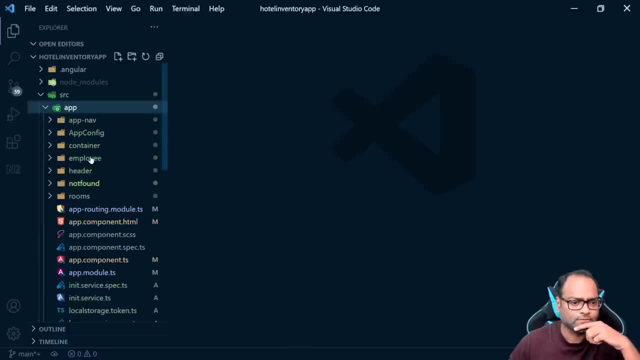 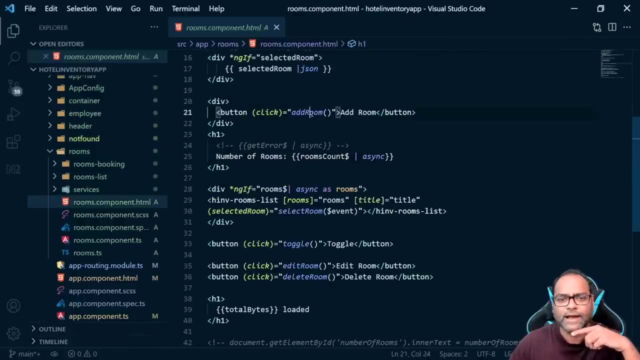 So, first thing, we already, uh, have some functionality available, So let's close all of this. rooms? Uh, we have rooms list And, if you remember, we had this add button somewhere: add room. So what we need to do is we need to take this add rule functionality out and put it in a different component. 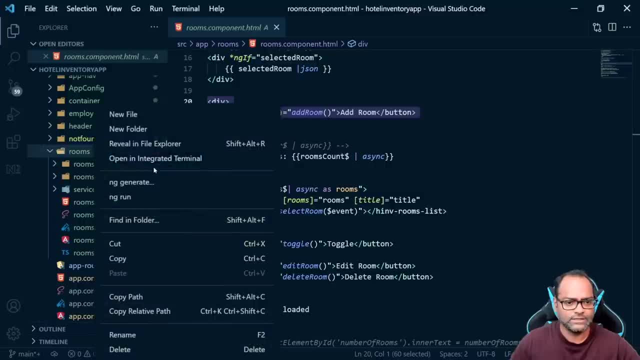 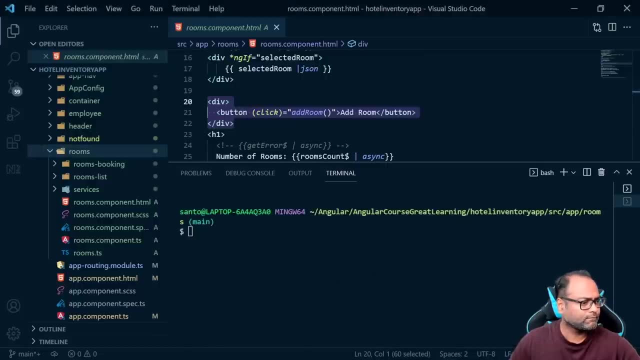 So what I'm going to do is I'm going to call it as A new component. So let's say: open an integrated terminal, And here we'll say NGGC and let's call it as the rooms Add Right. So it's uh, it will be used to add a new room. 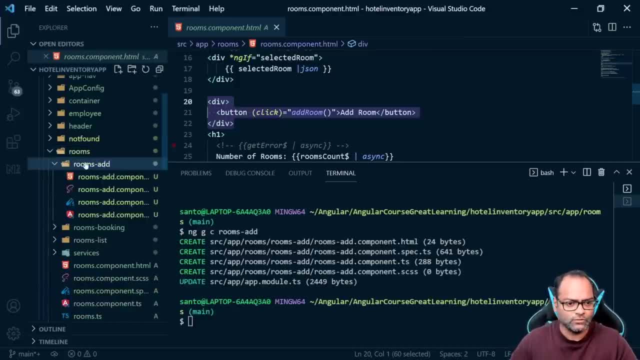 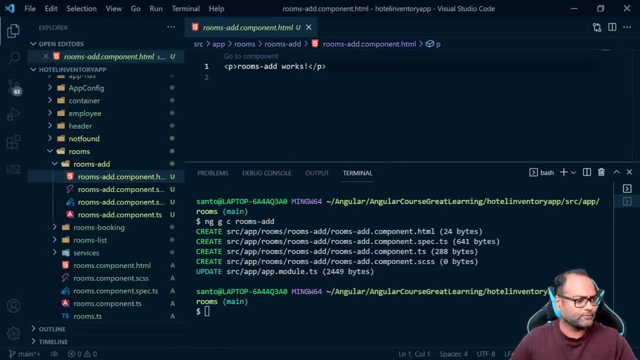 That's what we are planning. We're trying to To uh and let's see. So we got our component and let's go to the uh slides. right, Let's go to the slides and let's see what are the steps which needs to be performed. 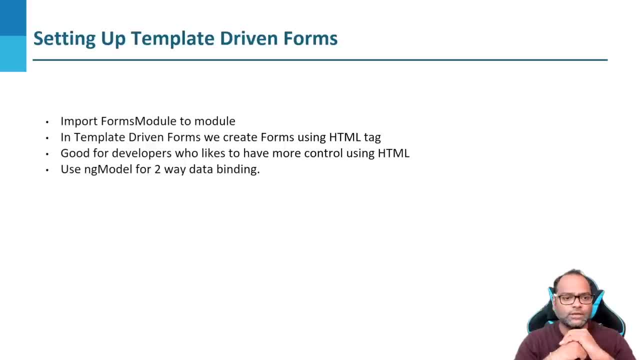 So first we have to add forms module to module and then we have uh, we have uh template driven forms. So that's next step. So how we create the forms, we'll come back to this. first Let's do the first step. 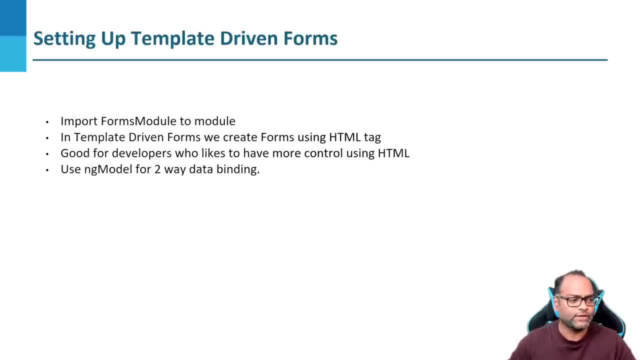 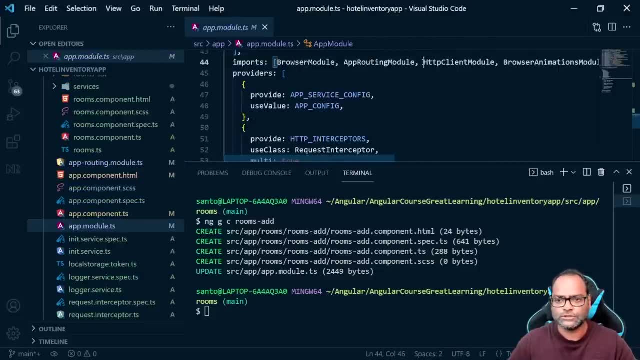 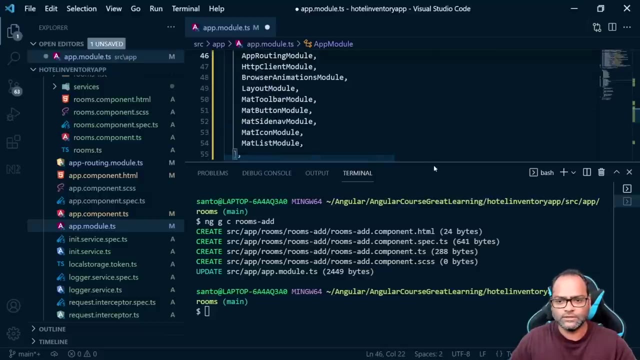 So first, import forms module to module. right now We have one module, So let's go ahead and add this to this module and into imports that it has. It's a module, Remember- and let's format with prettier and add forms. 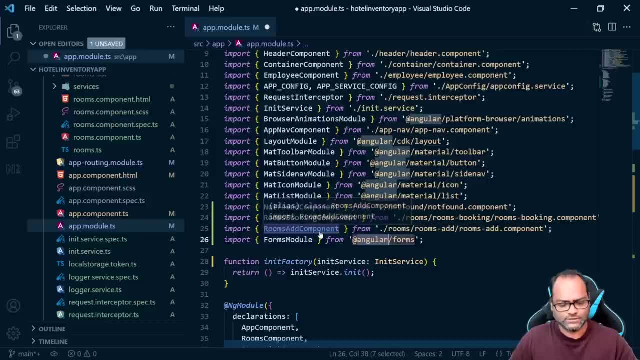 And it is auto imported for me, So from angular slash forms, and this is what you want you to do. Now let's go ahead and create a form. So, to create a forms, We, uh, we will be using HTML forms. 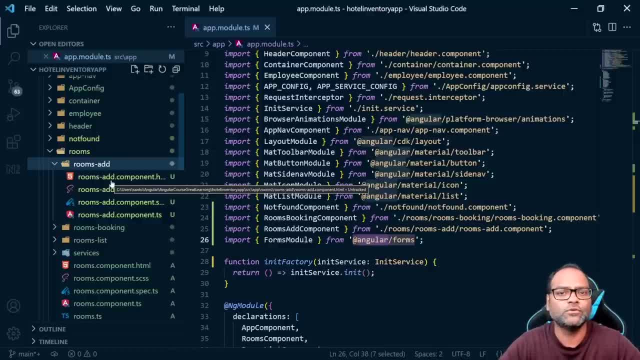 So we will be writing HTML form. You don't have to do something extra here. I mean, if you know HTML, you know how to create a form in HTML. That's what is needed to create a form in template driven forms. 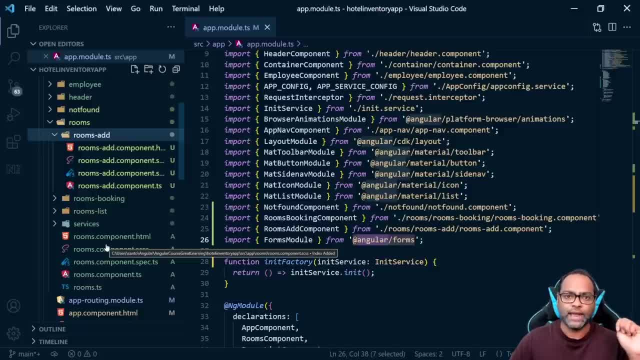 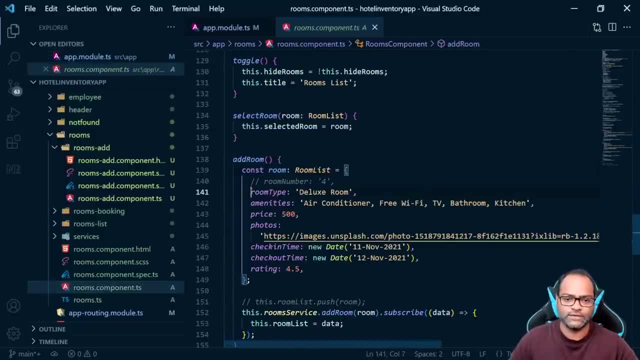 So let's first see what are the values which is required to add a book room, And for that we already have this add room functionality. So we need room type, We know, we need amenities, We need price, We need photos And check in time, check out time rating. 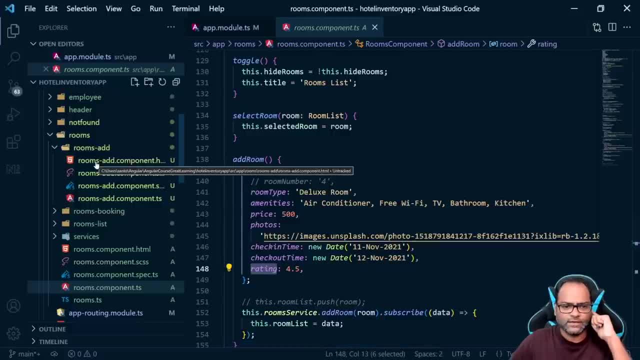 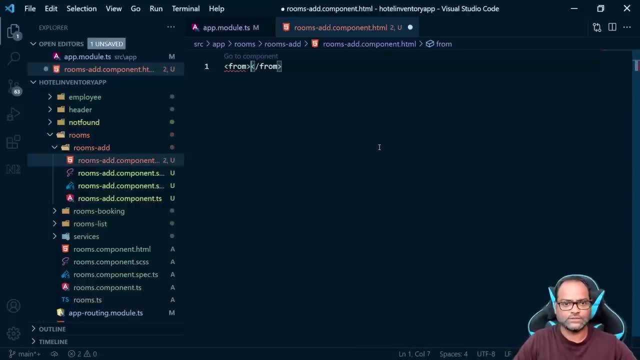 Right. So these are the things which we need. So let's go ahead and add a form for this. So I'm going to add form right. So this is, uh sorry, not from form right. So this is how we create a estimate form. nothing fancy, yet. 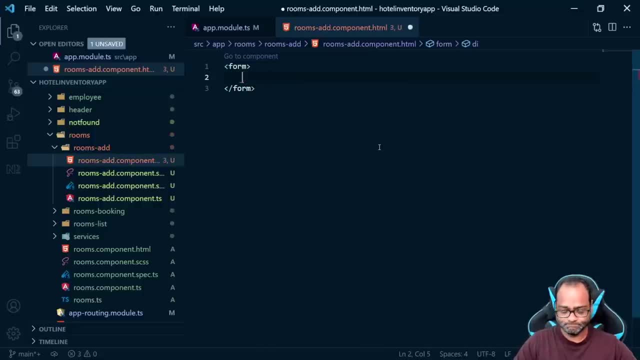 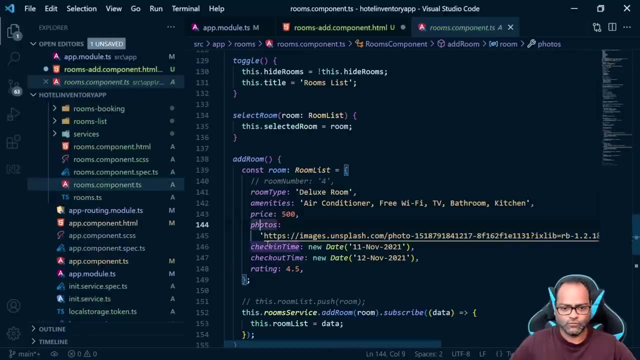 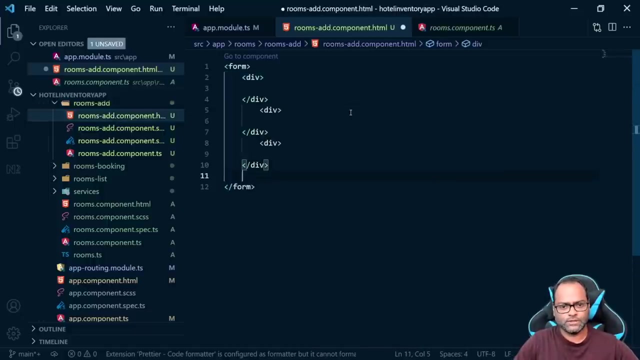 And let's add some divs. Let's see how many fields we had: One, two, three, four, five, six, seven. So I'll add seven divs: The four, five, six, seven, and I will add one more for submit button. 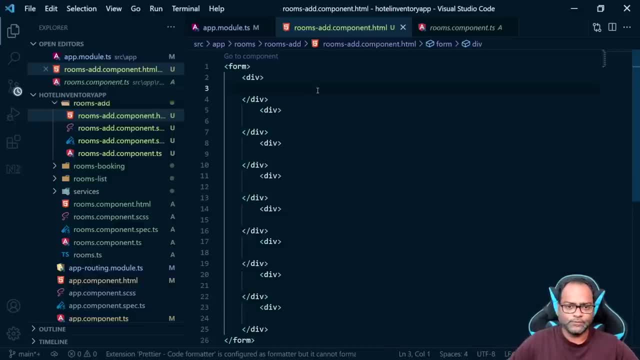 So it, that's it. And now here, uh, we I'm going to use some bootstrap classes. So, uh, bootstrap has something called, uh, form group, So let's use form. So for all the divs, we can use form group. 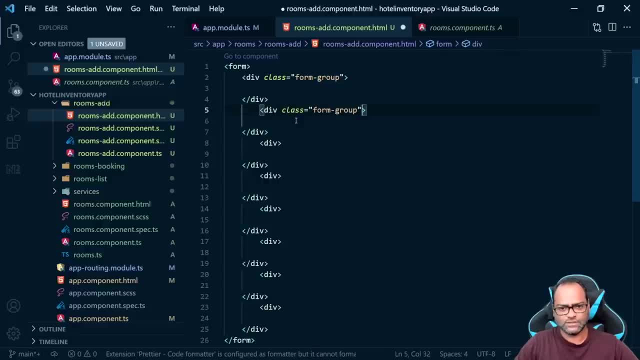 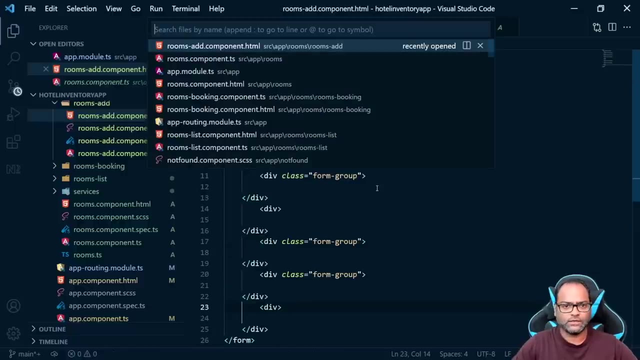 What it will do. it will just add some space. So that's what it is going to do, Except the last one, because, um, that will be our submit button, So that we already, uh, get so form group, and now we need controls. 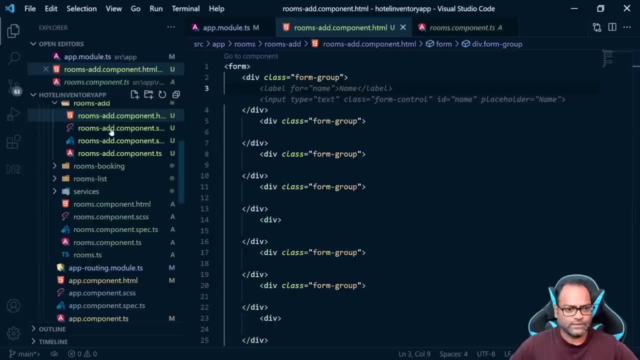 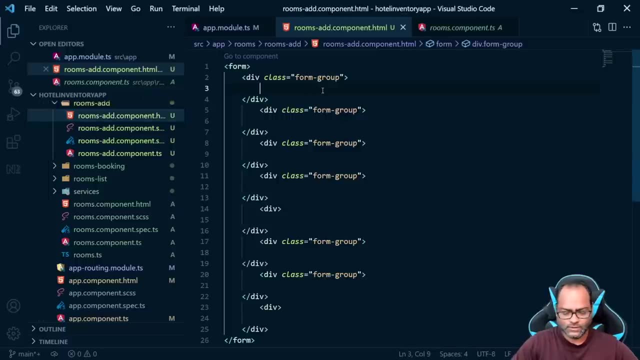 We need, uh, our controls to be added, So Let's go ahead and do that. So we have room type. So I'll say input and we have to say type Uh. so input, uh type will be text and name. 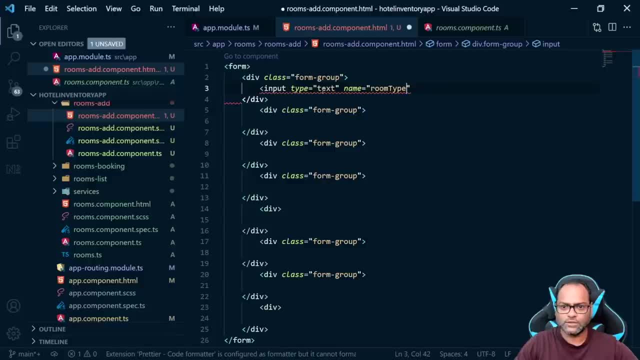 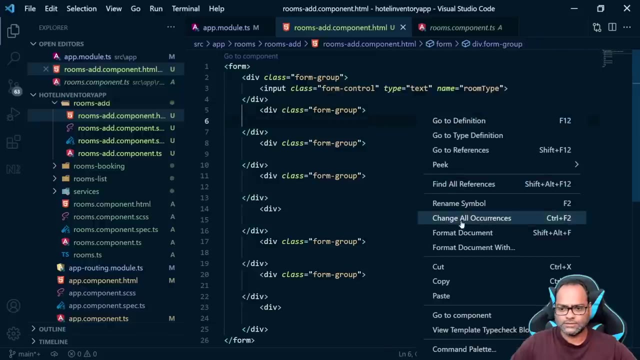 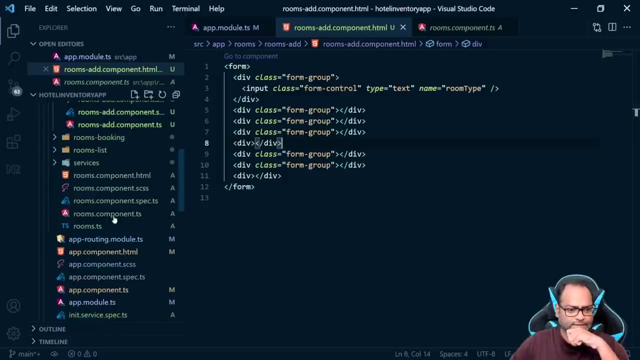 Let's give a name, uh, which will be not room type, And here we are going to use a class of type, Form control, And let's format the document So, uh, what we will do is we will create a route for adding up room. 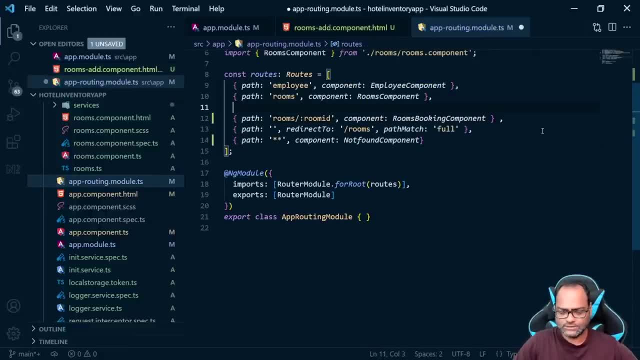 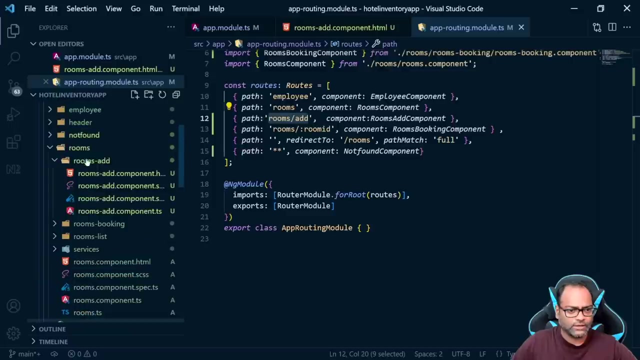 And let's go ahead and do that here. So here I'll just add path. We'll say, uh, it's rooms, slash, add and component. And we'll say, uh, we need to add this into our routes. uh, sorry, our navigation bar. 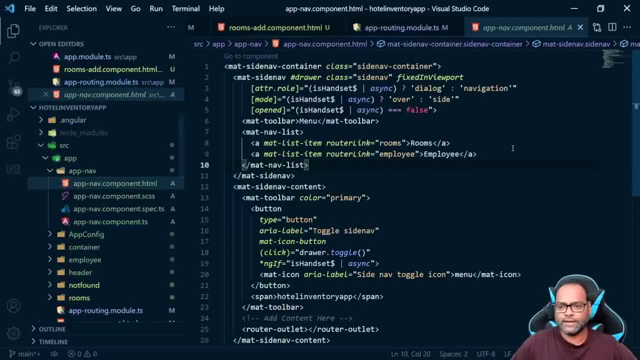 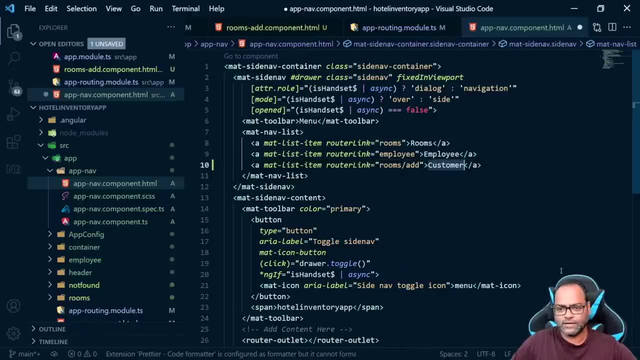 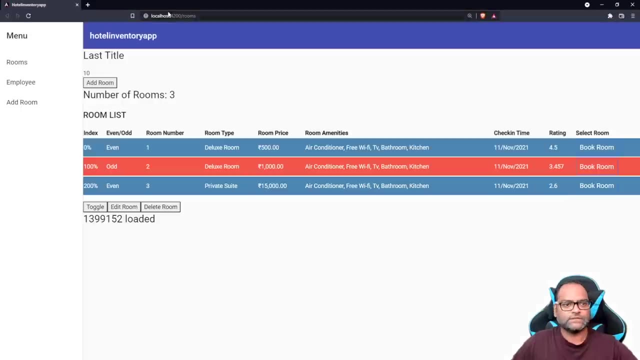 So let's go to network, go to HTML, and here we will add Outlink to rooms, slash add And we'll say add Room. Let's verify this functionality first. Let's say add room and we have this input text available here. 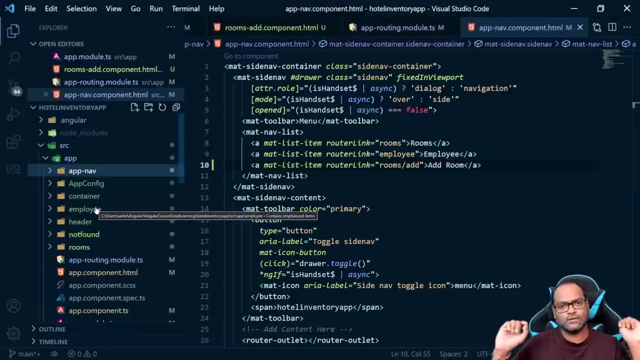 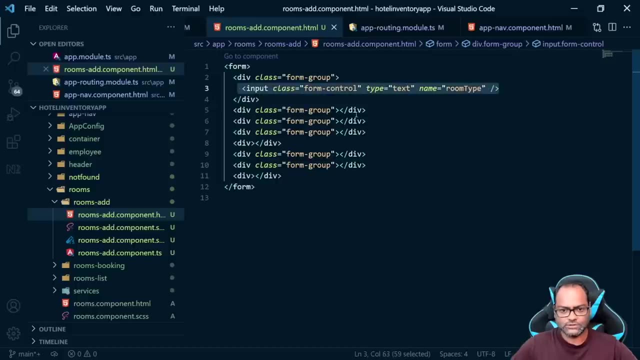 So first step is done. We um added a forms module. We just created an input field, We added a uh route, That's it. And now let's complete that form. So let's go to rooms, slash, add and let's add the other inputs. 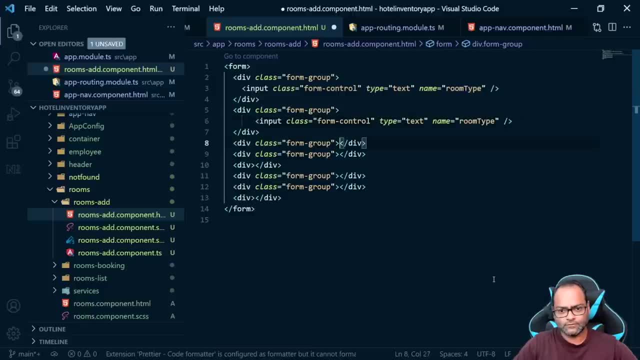 So we can see, uh, we can see that our ArrayList actually has a couple of is said to be available. You know, if you have a group that doesn't have an array of our ArrayList and we're going to add it to a group for our groups, uh, this will be suitable for those groups. 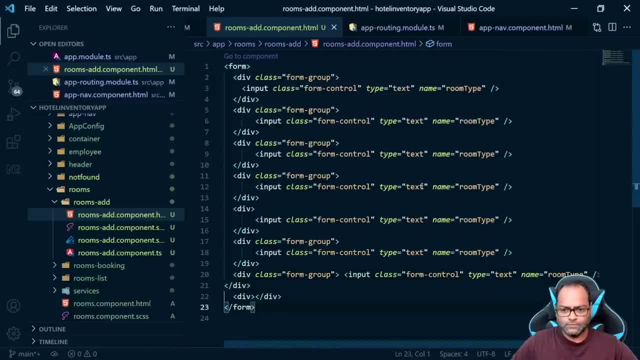 So let's go ahead and do that. I'm going to do that by selecting a group. You can see the group name. It's just a little bit, That's all. So let's go ahead and do that. So let's go ahead and do that. 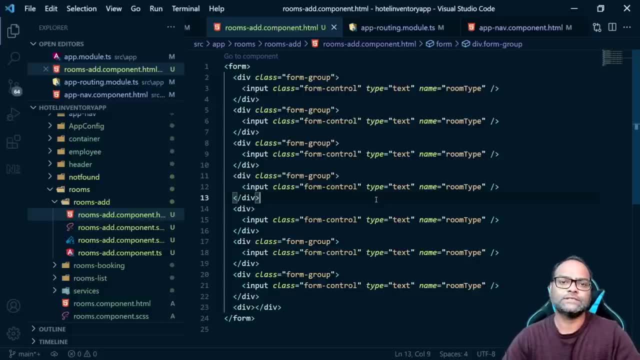 more about forms. why we create forms. remember, in case you have an enterprise application, there will be some use cases where you have to collect user input. so that's the that's the reason you will be using forms mostly. for example, let's say, you have some filters which you need to show you. 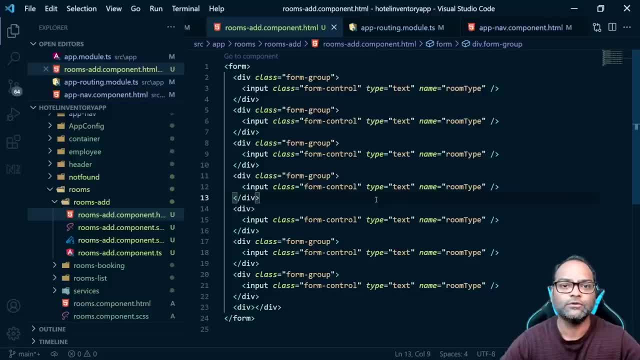 need to collect some user input in forms of feedbacks. you need to collect user profile information, that these are some cases where you may need forms. it's not mandatory, right? you can still have an entire application without forms. what are the use cases? like the, the applications. 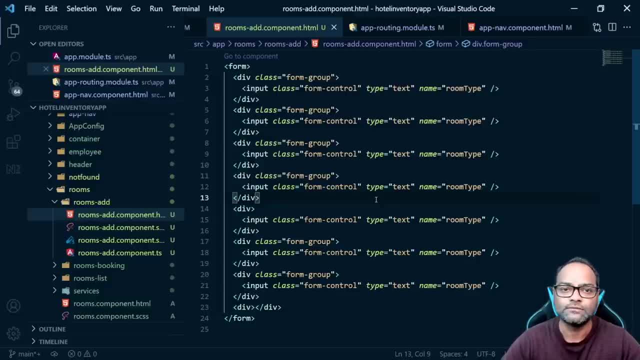 where you just need to display the data. for example, you have internal revenue system and uh. so what you will end up with so some charts and all those things, but still, you may need some filters as well, so that those are the scenarios where you will be using forms, and let's uh move. 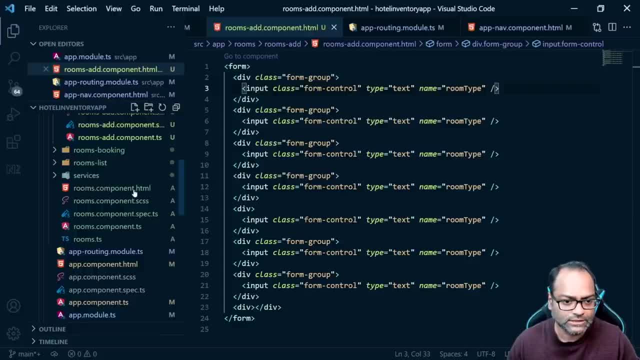 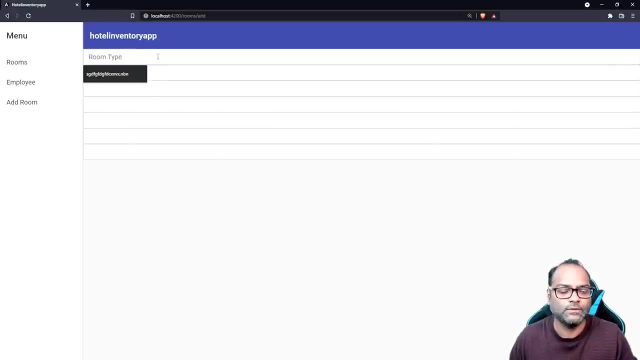 now and let's add other controls. so i'll say: this is, and we can add uh, one more thing, because we can add placeholder, so we know what we are, we are supposed to enter right. so i'll say: this is room type and let's see, so you have a nice uh placeholder available here. so it depends so a lot. 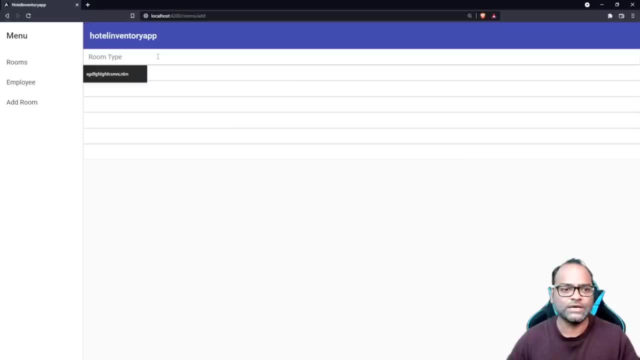 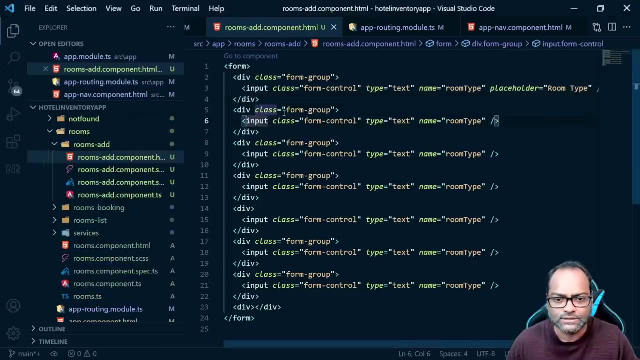 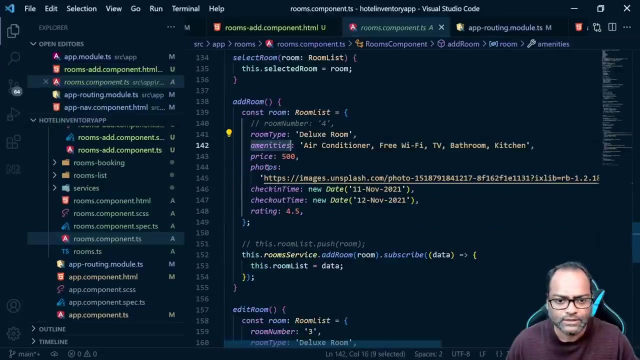 of applications uses label, but a lot of mobile first applications does not use label. they use placeholder. so it's up to uh, your design system how you want to proceed with it. so, and what we will do is let's see if i can add: um, okay, let's, uh, let's take css later and let's see what else we have here. amenities: 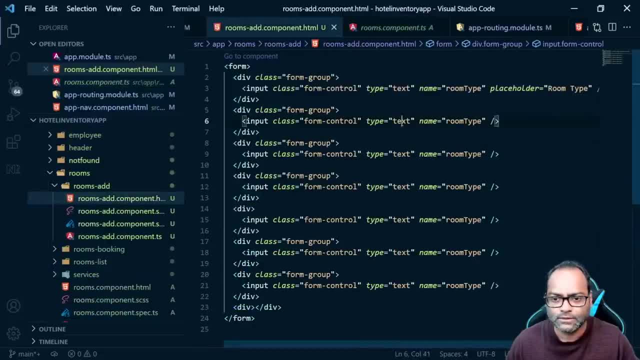 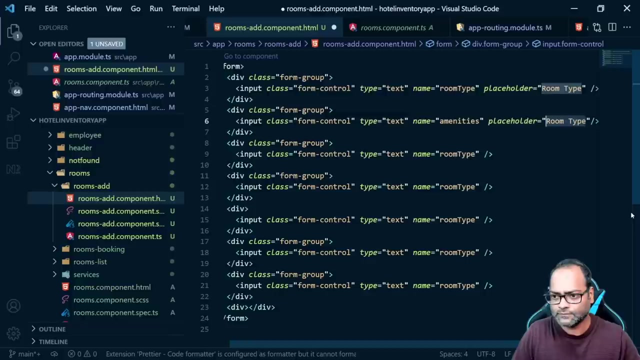 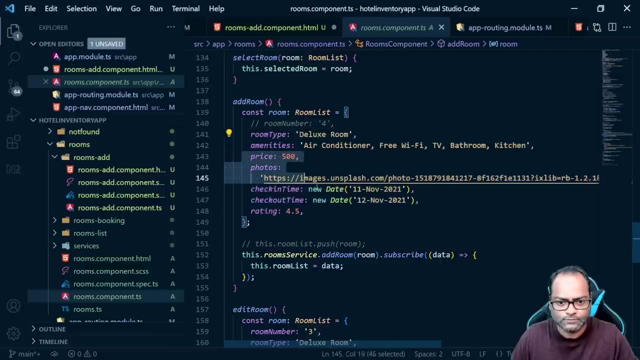 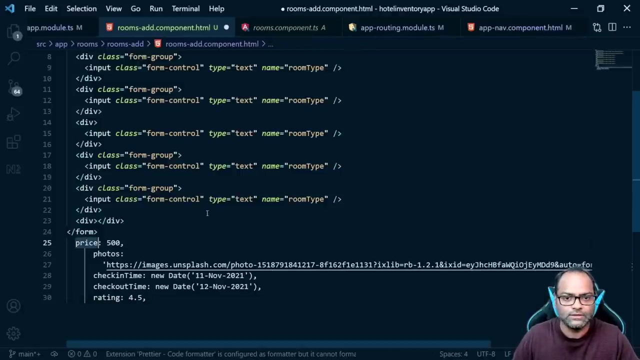 prices, photos, so amenities. so it will be, let's say, this will be text as well, and this will be these, and placeholder will be just a surprise. yes, i can just refer quickly. so let's see, this is input type, this is price, so is to say type is not. 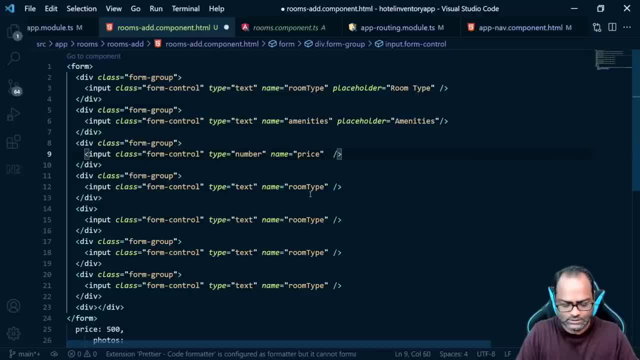 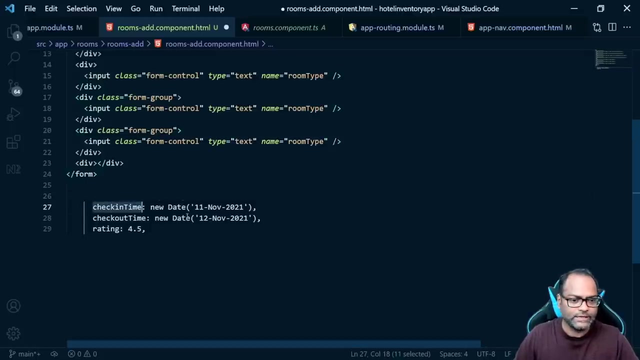 price and say this is placeholder room price per night, so because most of the prices are per night, then we have photos and this should be text and placeholder photos and we can say provide link. right, so this is done. and we need check-in and check-out time. so this is our date time, right, so we can. 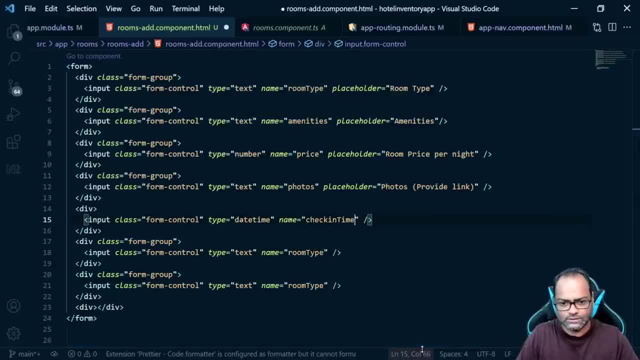 actually use date time and let's say check-in time and placeholder, because all the hotels actually have a date time. so we can actually use date time and, let's say, check-in time, have a check-in, check-out policy, right? so you have to check in by three. i mean it can be part. 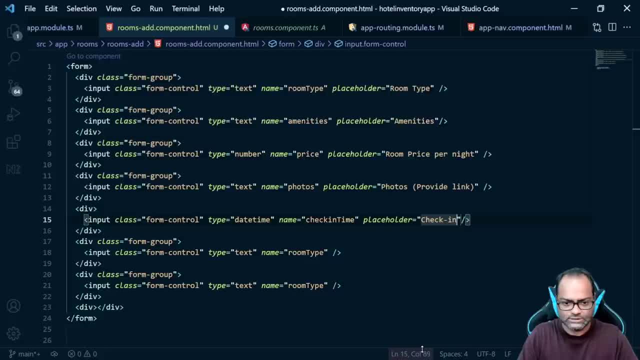 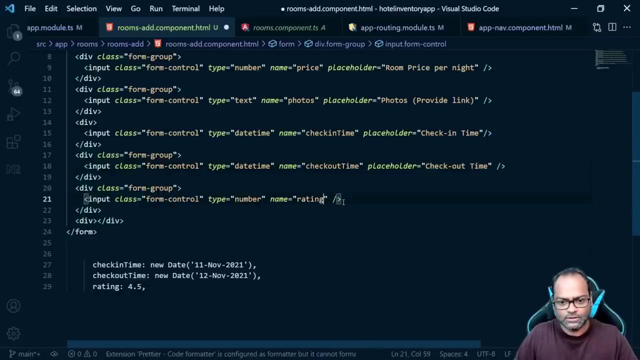 of policy, but let's try to keep it minimum. so i'll say this is check-in time and check-out time and this will be date time as well, and i'll say this is placeholder and this page about time and this is rating, so it will be again number rating. 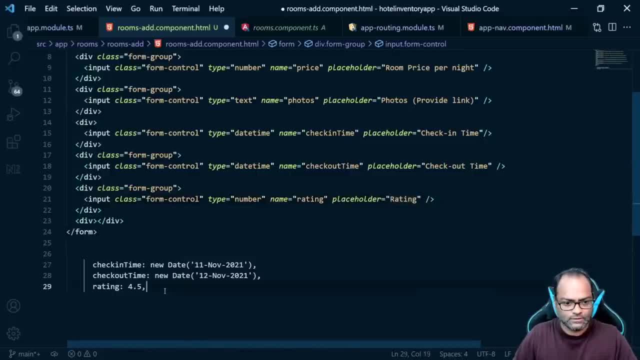 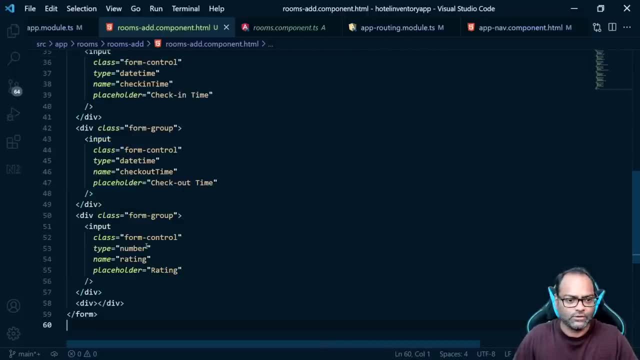 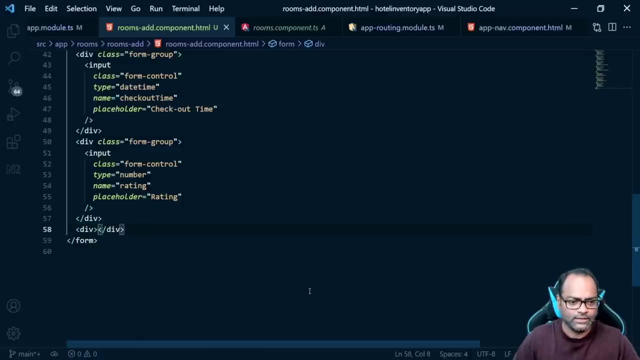 and placeholder also rating. you can in future actually replace this with some rating component. in case you come across some component library which has rating system or rating component, you can use it and here i will say button: okay, so we'll have a submit button available here. so you have button, button, button, primary submit. 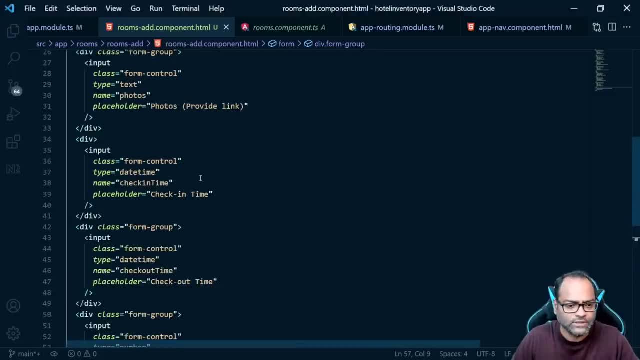 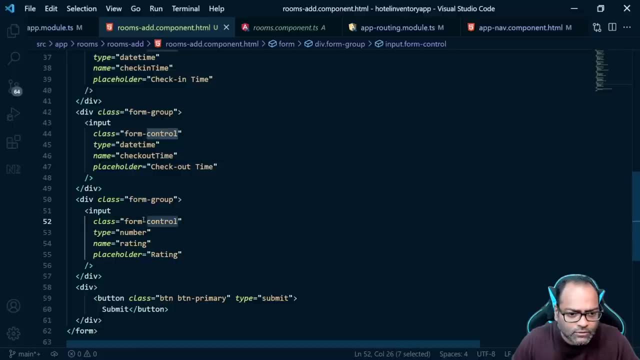 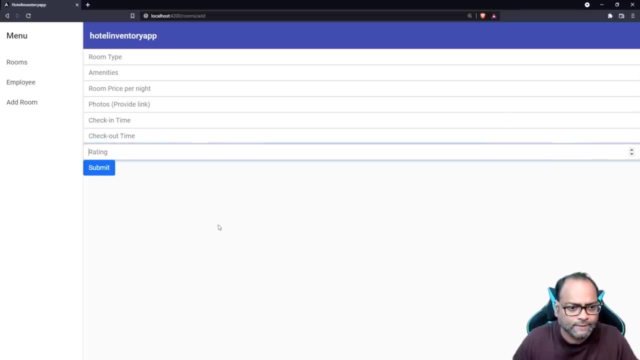 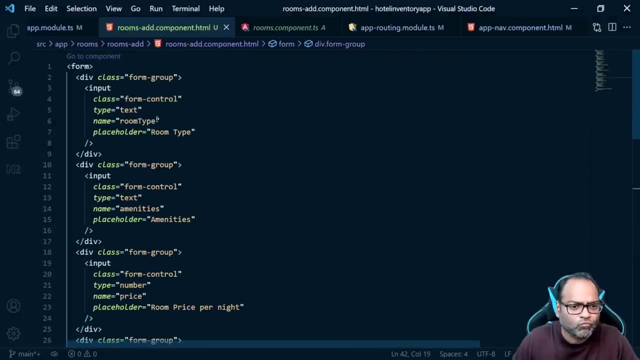 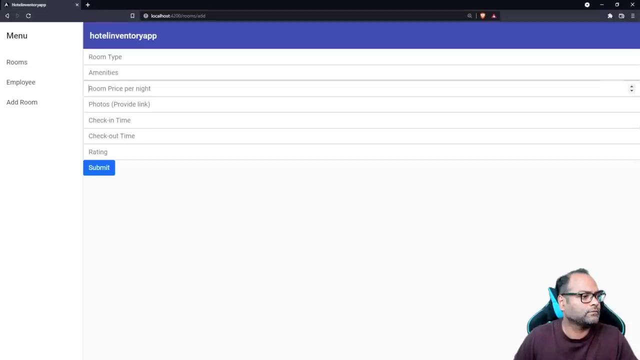 let's go ahead and verify forms. okay, this looks nice. i think there's some things which is missing form, but class form control form group. we thought this was actually in button: form control group. right here is the feed mark. okay, so let's go and copy thisand we'll need this. 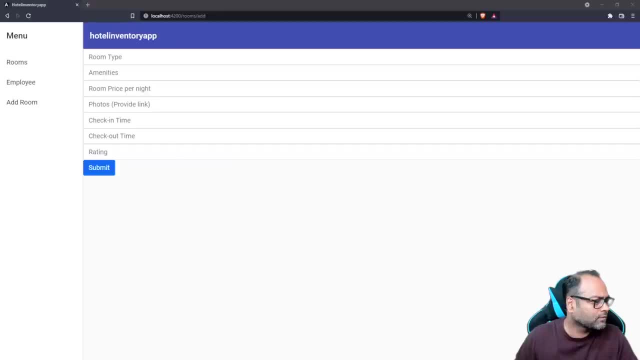 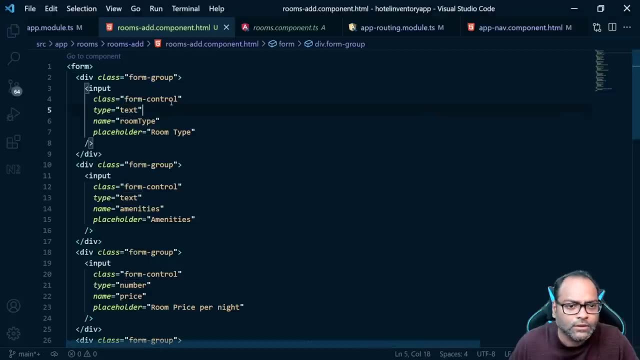 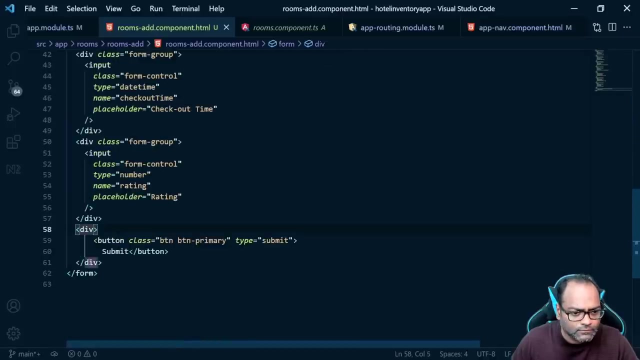 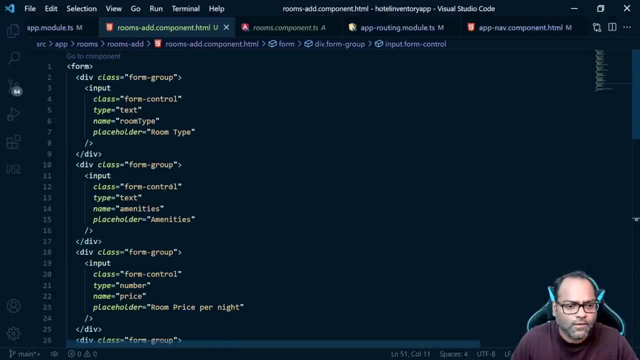 file, so i'll use this as a departure document. okay, so i think the spaces are missing. let me verify class form group again. this is correct. some control. this is too much. okay, so now we have this form available, but let's see, uh, let's see, uh. 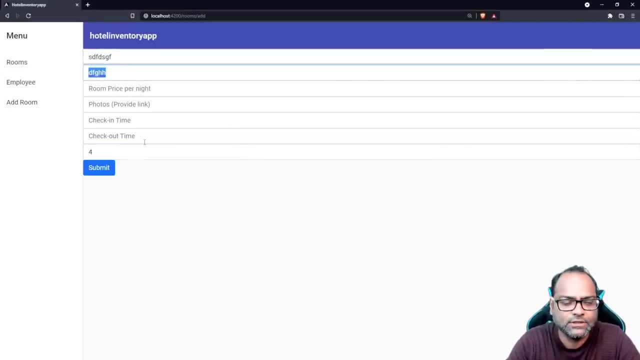 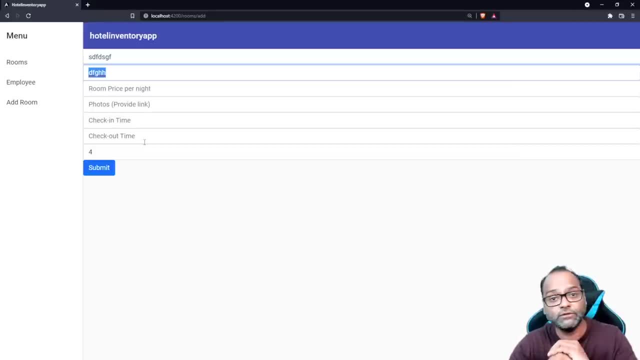 what's that? so we need to collect this information and send it to our back end information and send it to our back end information and send it to our back end. that is something which is missing. how that is something which is missing. how that is something which is missing. how we'll do that. 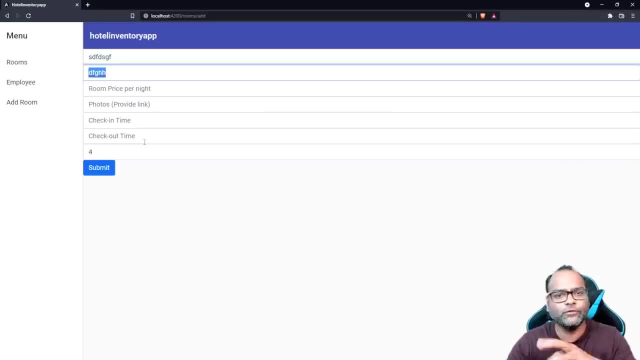 we'll do that. we'll do that so to do to achieve that. we need some so to do to achieve that. we need some so to do to achieve that. we need some two-way data binding, which is uh which. two-way data binding, which is uh which. 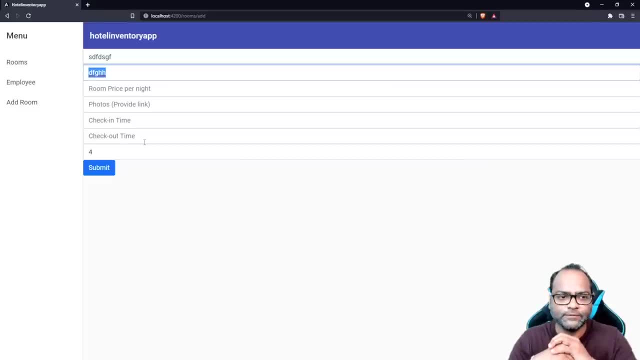 two-way data binding, which is uh, which needs to be, needs to be, needs to be available. how we do two-way data binding available. how we do two-way data binding available. how we do two-way data binding. so angular forms provide it by default. so angular forms provide it by default. 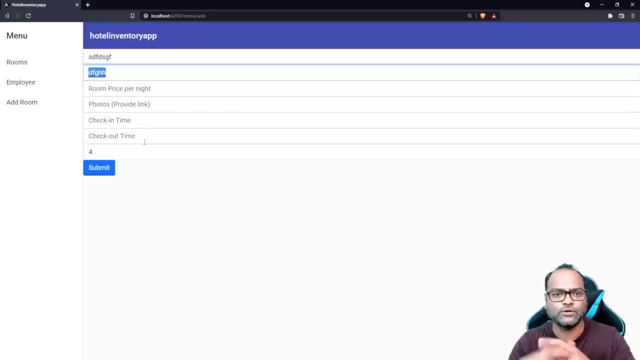 so angular forms provide it by default. so in case you want to do it, do two-way. so in case you want to do it, do two-way. so in case you want to do it, do two-way. data binding: we will discuss about what. data binding. we will discuss about what. 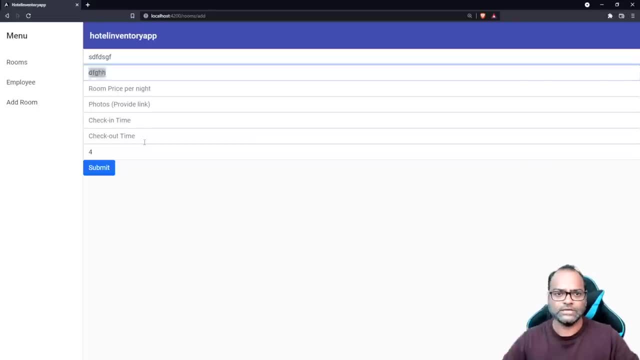 data binding. we will discuss about what two-way data binding is. two-way data binding is two-way data binding is: uh, but let's see it in picture. and then uh, but let's see it in picture. and then uh, but let's see it in picture, and then we'll, we'll do that. 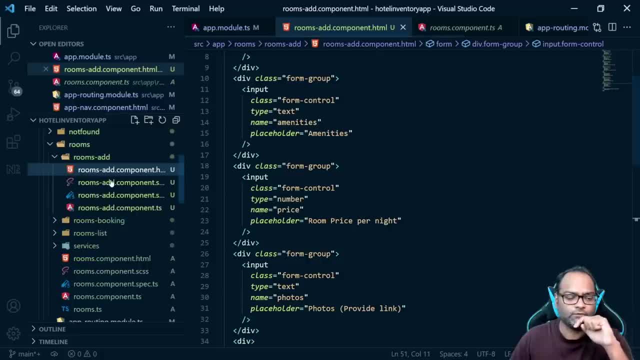 we'll, we'll do that, we'll, we'll do that. so, first thing, uh, we need a model. uh. so, first thing, uh, we need a model. uh. so, first thing, uh, we need a model. uh, what we uh, the model which we are, what we uh, the model which we are. 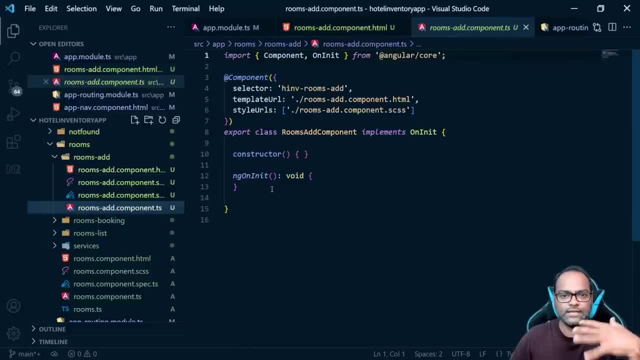 what we, uh, the model which we are talking about, is we need a talking about? is we need a talking about? is we need a interface which tells us how my interface, which tells us how my interface, which tells us how my room information is going to look like? 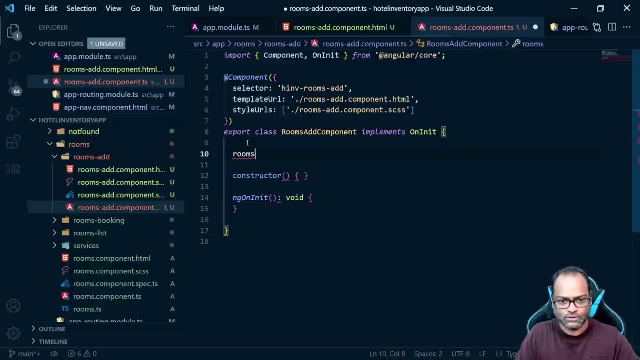 room information is going to look like. room information is going to look like: so to do that, i will create a room. so to do that, i will create a room. so to do that, i will create a room which is type of, which is type of, which is type of. let's see room. 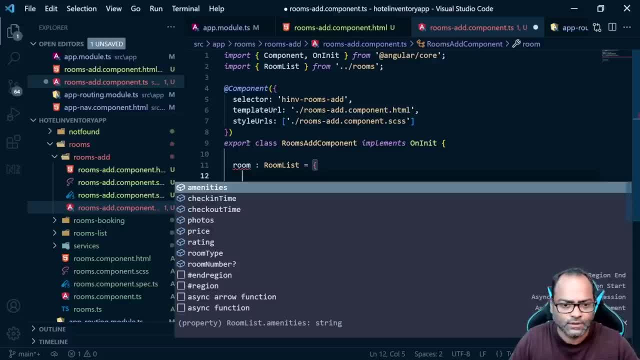 let's see room. let's see room list. i think list, i think list. i think is equals to, is equals to, is equals to. yeah, this is the uh, so remember id room. yeah, this is the uh, so remember id room. yeah, this is the uh, so remember id room number. we have made uh anyways, optional. 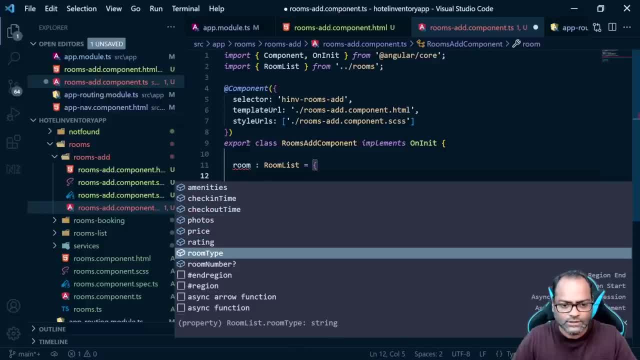 number. we have made uh anyways, optional number. we have made uh anyways optional. so let's, so, let's, so, let's add some uh other things. so it's a room, add some uh other things. so it's a room, add some uh other things. so it's a room type this: this will be the default. 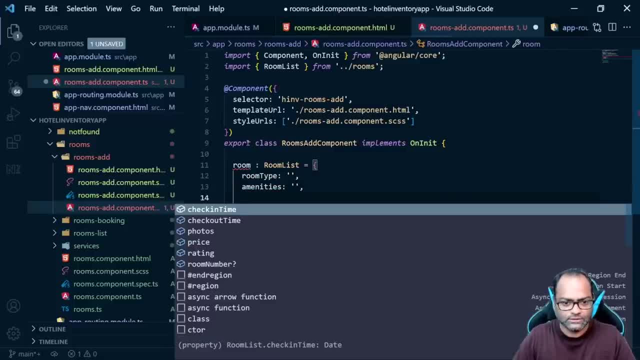 type this. this will be the default type. this. this will be the default values which we are adding right now. values which we are adding right now, values which we are adding right now: amenities, amenities, amenities and check in time and check in time and check in time. check out time. 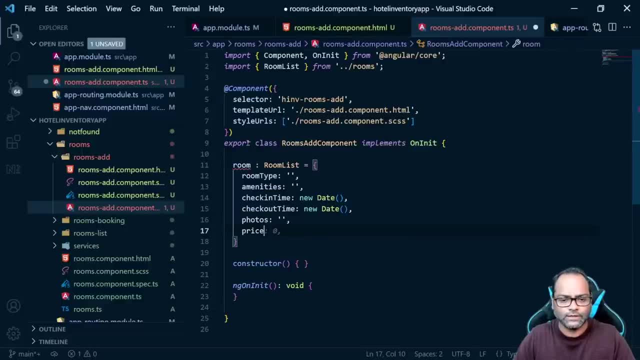 and then we have photos, and then we have photos, and then we have photos, we have price, and then we have rating, we have price, and then we have rating, we have price, and then we have rating. so these are the default values whenever. so these are the default values whenever we are supposed to enter some values. 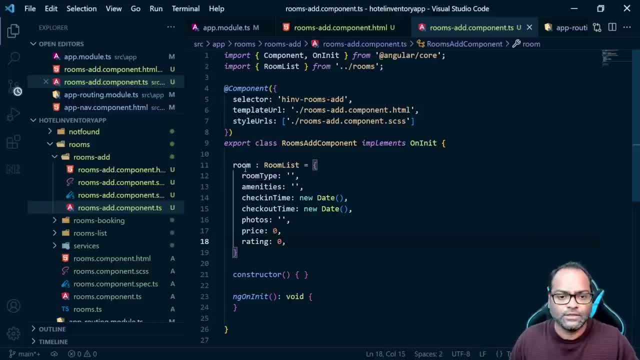 we are supposed to enter some values. we are supposed to enter some values into the form. this will be the default into the form. this will be the default into the form. this will be the default values which will be available, values which will be available, values which will be available. now we need to connect this. 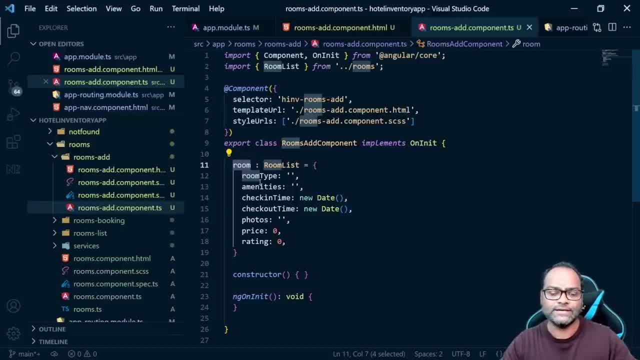 now we need to connect this. now we need to connect this model. like this represents our forms model. like this represents our forms model. like this represents our forms: fields right. so now we need to connect fields right. so now we need to connect fields right. so now we need to connect this model to our form so we can pass. 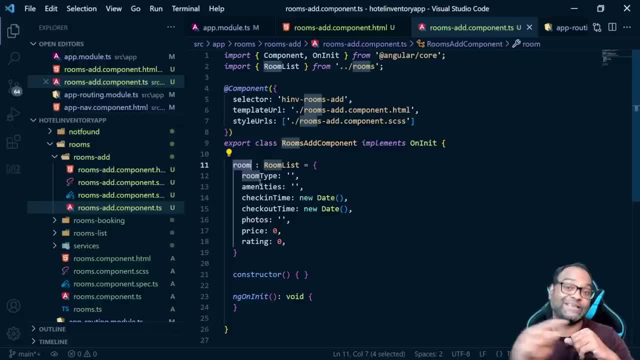 this model to our form, so we can pass this model to our form. so we can pass the information from template to my ts, the information from template to my ts, the information from template to my ts file and vice versa. even i, if i change file and vice versa, even i, if i change. 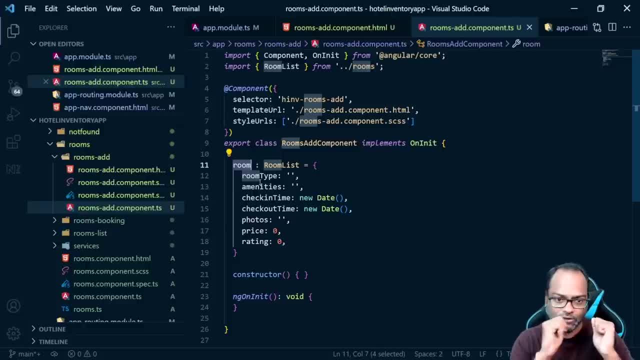 file and vice versa. even i, if i change something in my typescript file, it something in my typescript file, it something in my typescript file, it should reflect back into my form. so should reflect back into my form. so should reflect back into my form. so these are the. that's what we are. 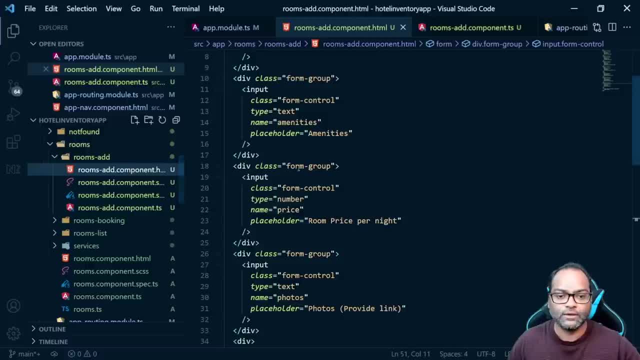 these are the. that's what we are. these are the that's what we are supposed to do here. so let's see how we supposed to do here. so let's see how we supposed to do here. so let's see how we can do that, can do that. 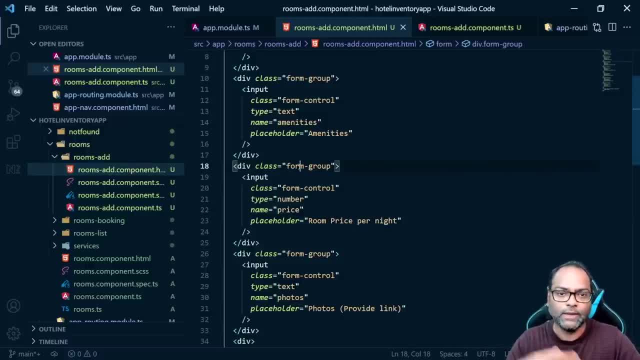 can do that. we have already added forms module into. we have already added forms module into. we have already added forms module into our, our, our module, so it it unblocks or it gives you module, so it it unblocks, or it gives you module, so it it unblocks or it gives you some functionality. what is those? 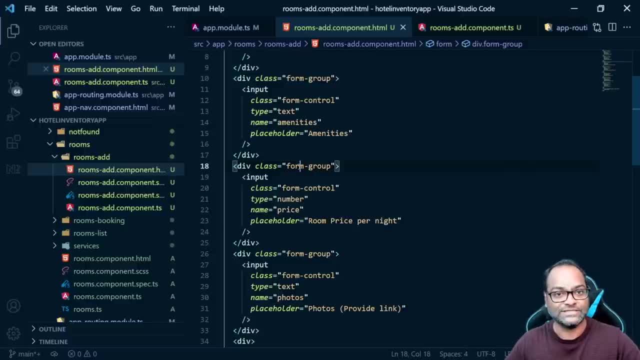 some functionality. what is those some functionality. what is those functionality, functionality functionality- it gives you info. functionality to it. gives you info. functionality to it. gives you info. functionality to achieved with data mining, how achieved with data mining, how achieved with data mining, how we have to use something known as. 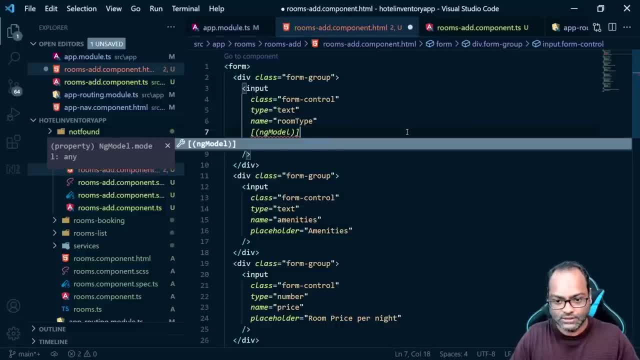 we have to use something known as, we have to use something known as ng model, so remember this. so you have ng model, so remember this. so you have ng model, so remember this. so you have to say ng model. to say ng model, to say ng model is equals to uh room. 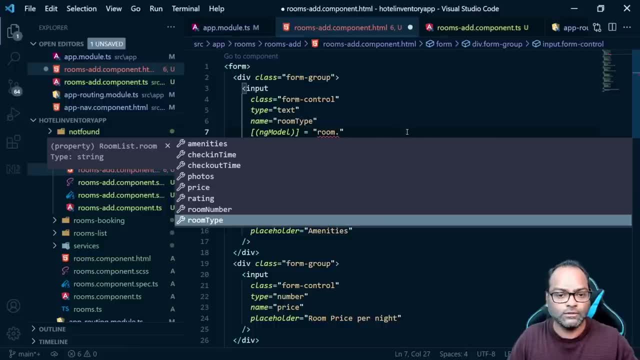 is equals to uh room, is equals to uh room, which is my property, which is my property, which is my property, dot, dot, dot, your, your, your, uh, sorry room, which is, uh, my model dot, uh sorry room, which is, uh, my model dot uh sorry room, which is, uh, my model dot property name. so here we are supposed. 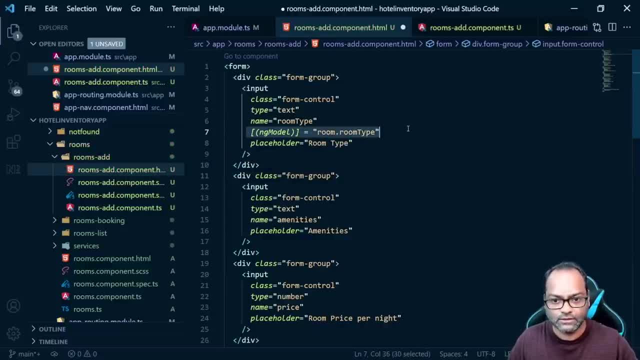 property name. so here we are, supposed property name. so here we are supposed to get room type, to get room type, to get room type right. so this is right, so this is right. so this is done here, done here, done here. let's add for others, so i'll say room. 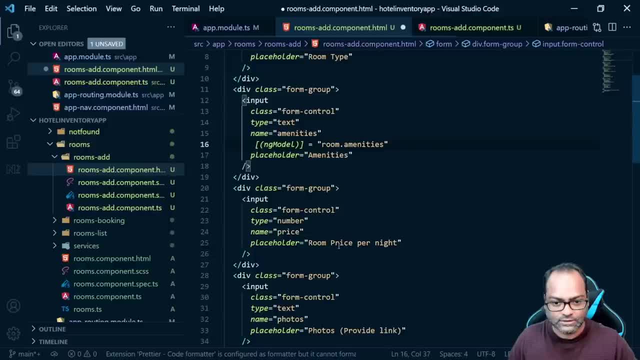 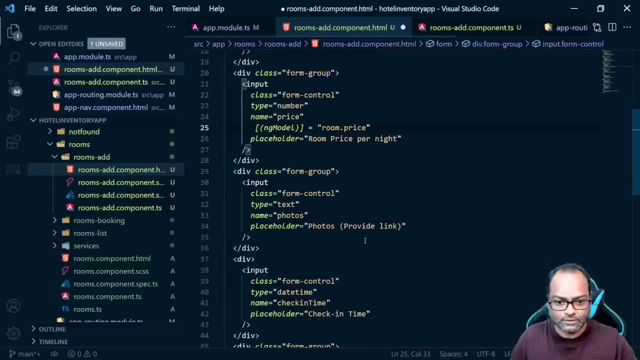 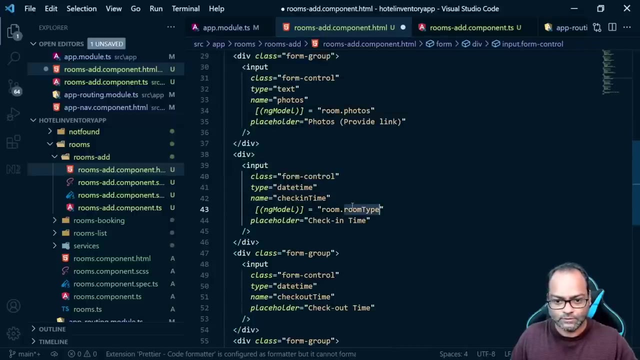 let's add for others, so i'll say room. let's add for others, so i'll say room type. this will be amenities type. this will be amenities type. this will be amenities. this will be. this will be. this will be price. this will be photos. this will be. 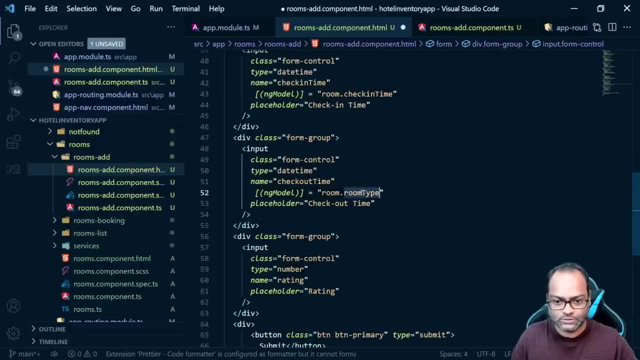 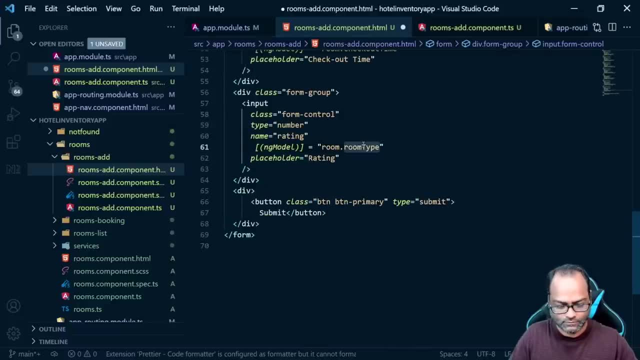 this will be. this will be check-in time: check-in time, check-in time. this would be. this would be: this would be checkout time: checkout time, checkout time. so so, so, and this will be rating. now, we added this: now, what, what next, how? now, we added this: now, what, what next, how? 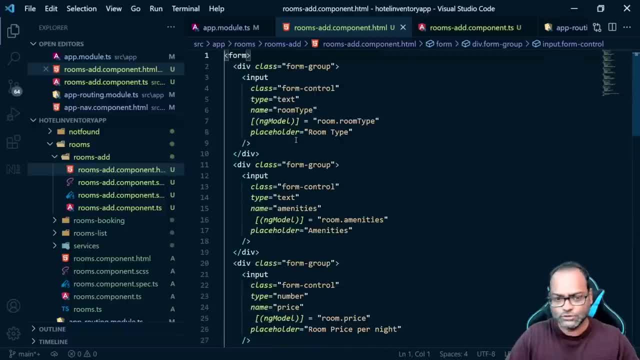 now we added this. now what? what next? how? we can verify that two-way data binding. we can verify that two-way data binding. we can verify that two-way data binding is working fine. let's see that. so what is working fine? let's see that, so what? 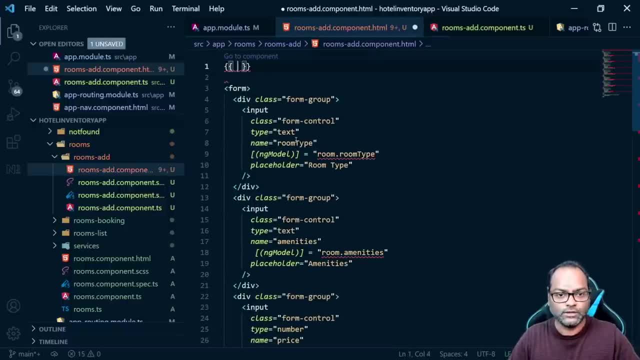 is working fine. let's see that. so what we can do is as room is my property. we can do is as room is my property. we can do is as room is my property, which is supposed to, which is supposed to, which is supposed to update whenever i enter some value, value. 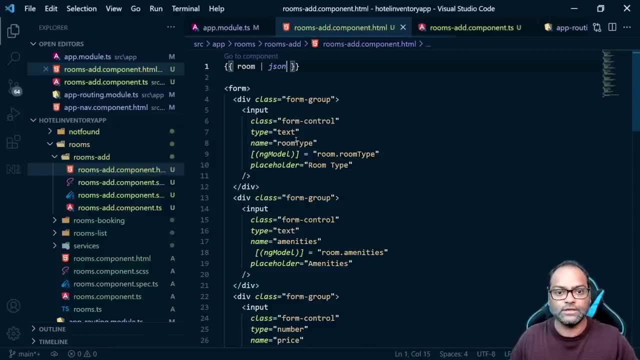 update whenever i enter some value value. update whenever i enter some value value. here i can just do something like this. here i can just do something like this. here i can just do something like this room pipe json, let's see and you can see, it has room type amenities. 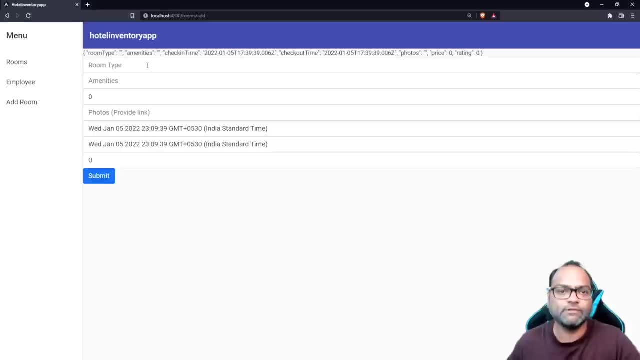 and you can see it has room type amenities and you can see it has room type amenities. check-in time checkout time photos. check-in time checkout time photos. check-in time checkout time photos. price rating: everything is available. price rating: everything is available. price rating: everything is available. let's add something in room type. you can. 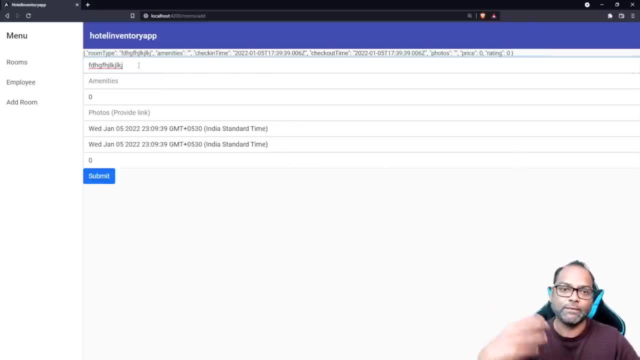 let's add something in room type you can. let's add something in room type you can see the value is getting changed. see the value is getting changed. see the value is getting changed. it means now i have the power of two-way. it means now i have the power of two-way. 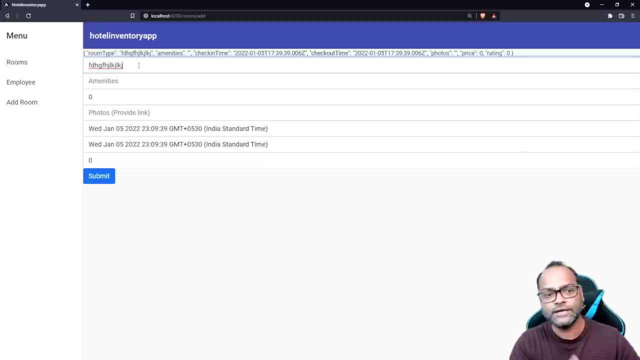 it means now i have the power of two-way data binding available. data binding available. data binding available with me. so whenever i make some changes with me, so whenever i make some changes with me, so whenever i make some changes here, it will be reflected back here. it will be reflected back. 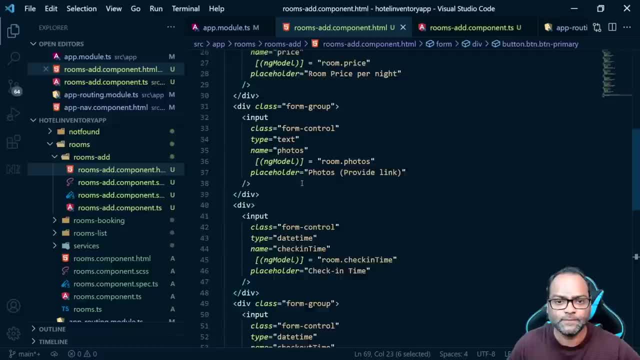 here it will be reflected back. done so? here we have a submit button. done so? here we have a submit button. done so, here we have a submit button. right, but how to submit this form? let's right, but how to submit this form, let's right, but how to submit this form? let's go ahead and do that. 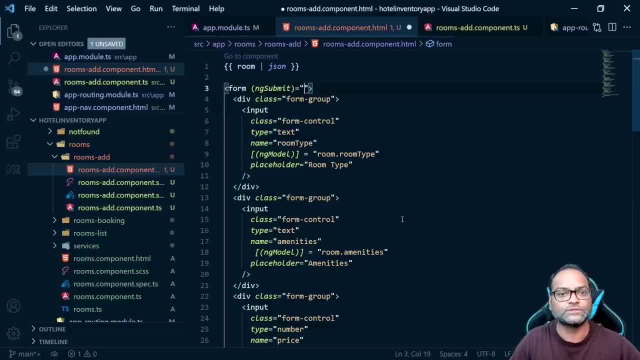 go ahead and do that. go ahead and do that. we can see uh ng submit is equals to a. we can see uh ng submit is equals to a. we can see uh ng submit is equals to a function which will actually add this function, which will actually add this. 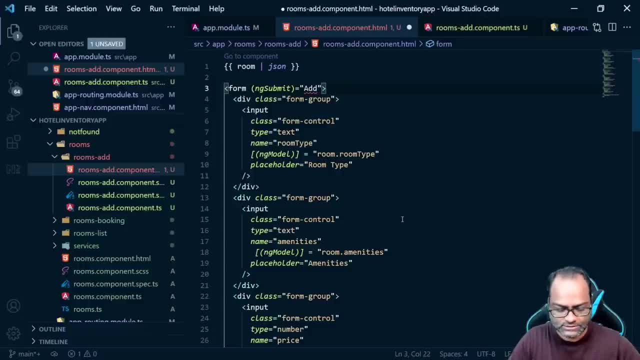 function which will actually add this data or send this data to our back end. so data or send this data to our back end. so data or send this data to our back end. so i can say this is add room function. i can say this is add room function. 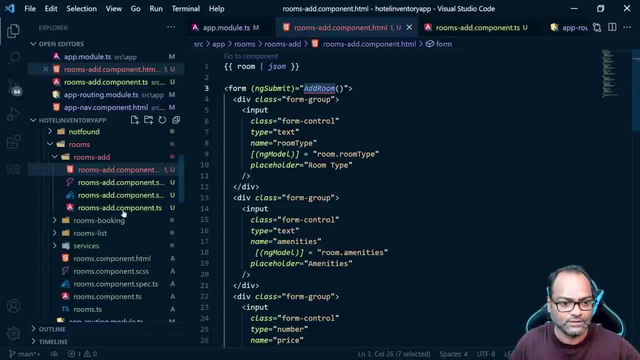 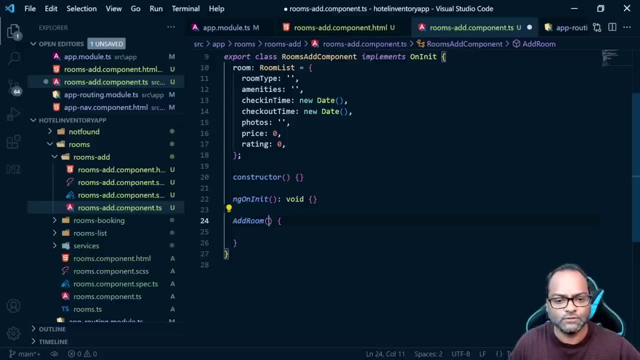 i can say: this is add room function, which we will implement, which we don't, which we will implement, which we don't, which we will implement, which we don't know, because we already have all the know, because we already have all the know, because we already have all the information available as part of this. 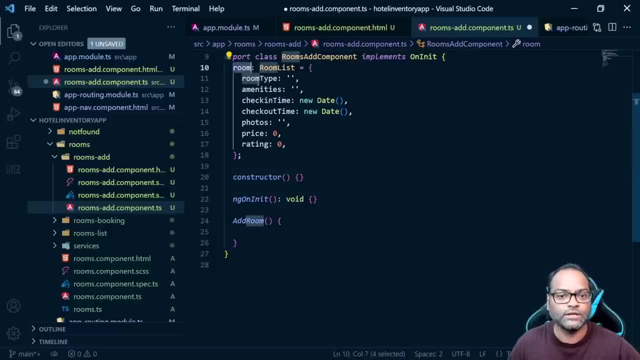 information available as part of this information available as part of this model, because whatever value we enter model, because whatever value we enter model, because whatever value we enter is updated into this property so we can is updated into this property, so we can is updated into this property so we can just do something like this. so 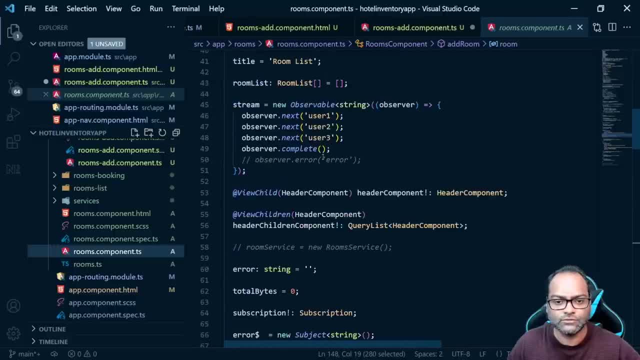 just do something like this. so just do something like this so i can go to room componentts. we need to. i can go to room componentts. we need to. i can go to room componentts. we need to get the reference to our service. get the reference to our service. 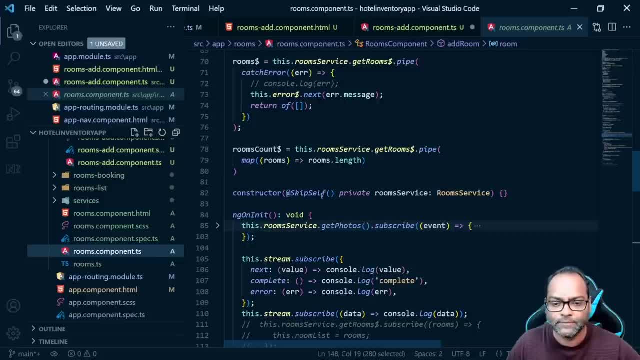 get the reference to our service, which is let's, which is let's, which is let's. where is the constructor yep this one? where is the constructor yep this one? where is the constructor yep this one? so i will say, uh, room service, i don't. 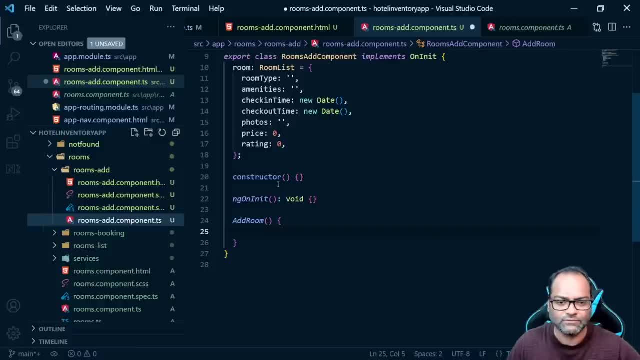 so i will say, uh, room service, i don't. so i will say, uh, room service, i don't want to want to want to. i can just avoid, skip self and all those i can just avoid, skip self and all those i can just avoid, skip self and all those things. because 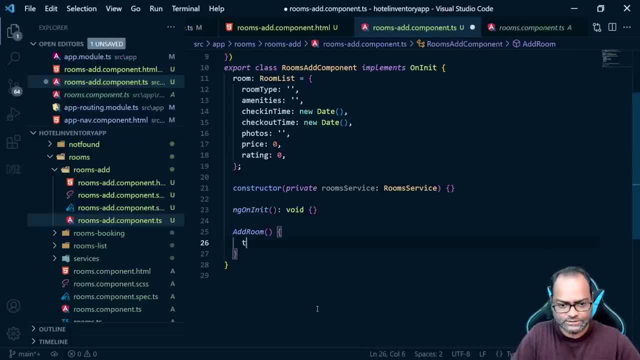 things, because, things, because we already discussed about it, and then we already discussed about it, and then we already discussed about it and then in add room: i can, we can do this dot in add room i can, we can do this dot in add room i can. we can do this dot. room surface dot. 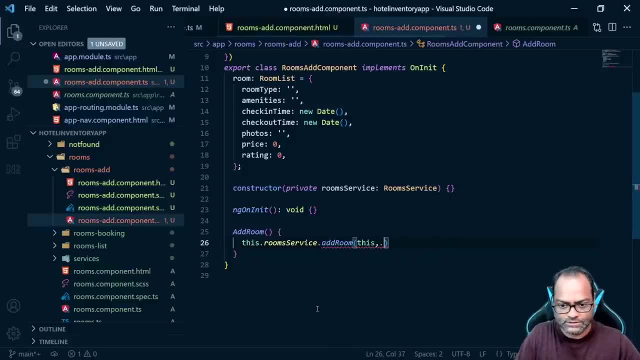 room surface. dot room surface. dot. add room. add room. add room: uh, where we can pass this dot room, uh, where we can pass this dot room, uh, where we can pass this dot room, and we'll subscribe. we'll say this is data and we'll subscribe. we'll say this is data. 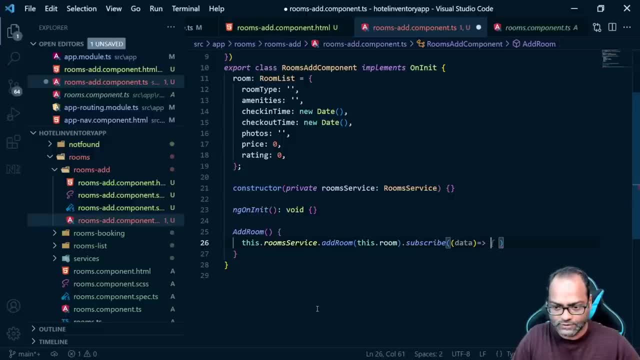 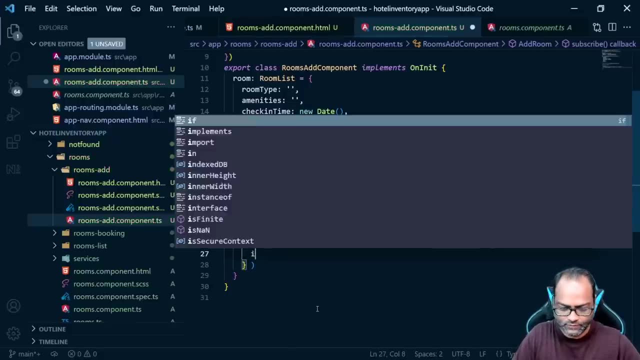 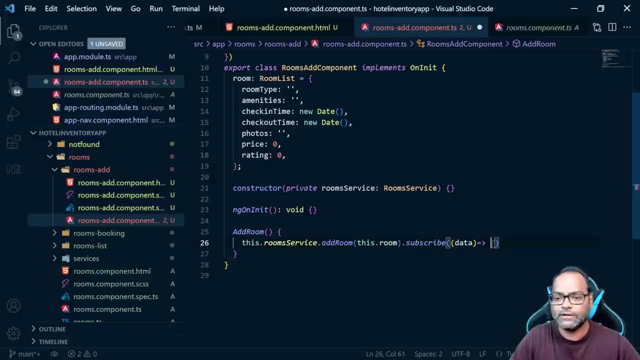 and we'll subscribe, we'll say this is data and and, and you'd say, if let's do something like if data dot, ah, okay, so right now we are in. ah okay, so right now we are in. ah okay, so right now we are in, we are actually giving all the data back. 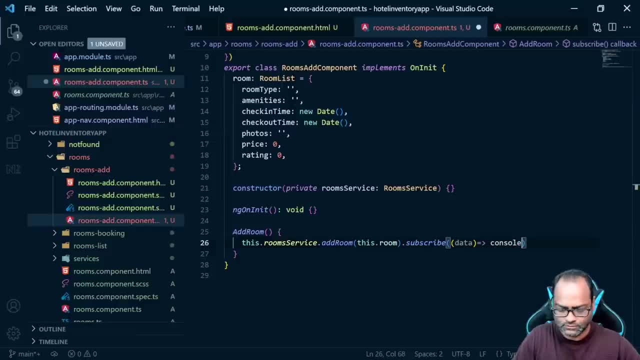 we are actually giving all the data back. we are actually giving all the data back. so we can just do something like this. so we can just do something like this. so we can just do something like this. i'll just do consolelog. i'll just do consolelog. 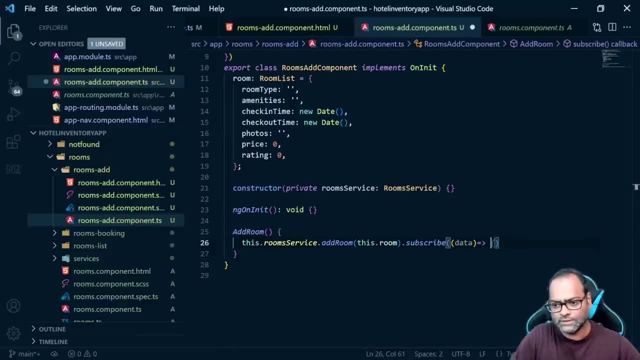 i'll just do consolelog. oh, let's do one thing, but one better. so oh, let's do one thing, but one better. so, oh, let's do one thing, but one better. so what we can do is what we can do. is what we can do is, i say, success. 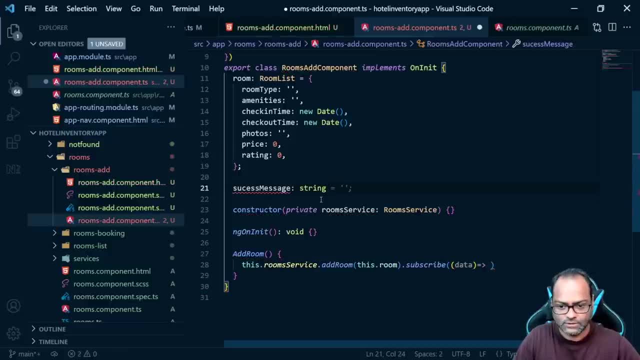 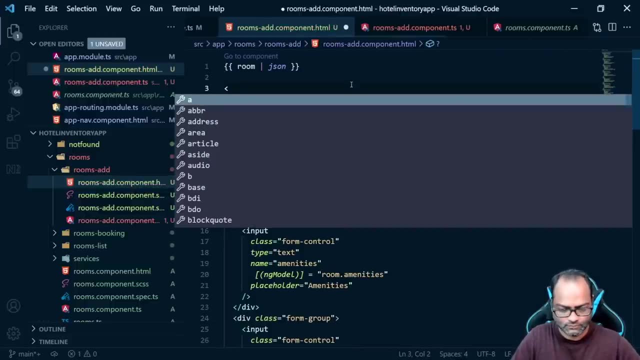 i say success, i say success, message, message, message, which is type of string, which is type of string, which is type of string is equals to this, is equals to this, is equals to this, and, and, and. you can add, you can add, you can add a div here. 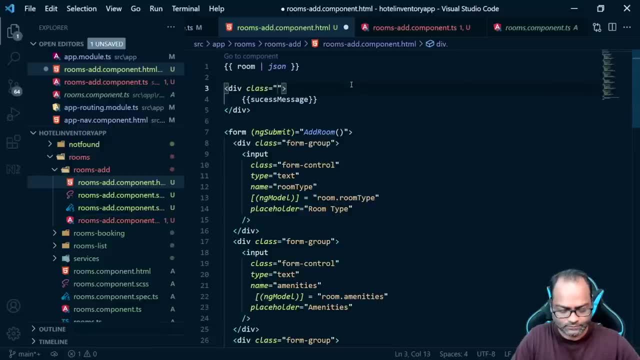 and we can add a class. and we can add a class and we can add a class strap. you can see which class we can use. you can see which class we can use. you can see which class we can use. right, we can use alert here, so you can. 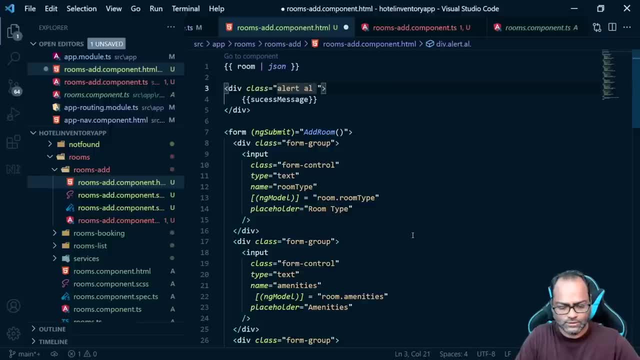 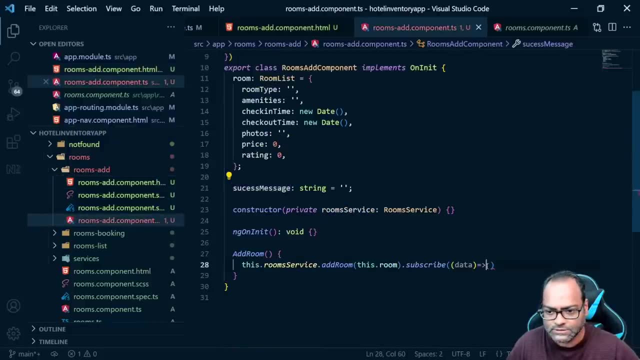 right, we can use alert here, so you can. right, we can use alert here so you can say: say: say alert, alert, success, success, success, right. and then we will set this message right, and then we will set this message right, and then we will set this message, i'll say this dot. 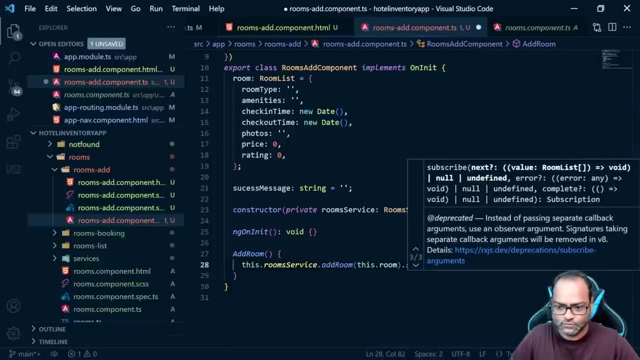 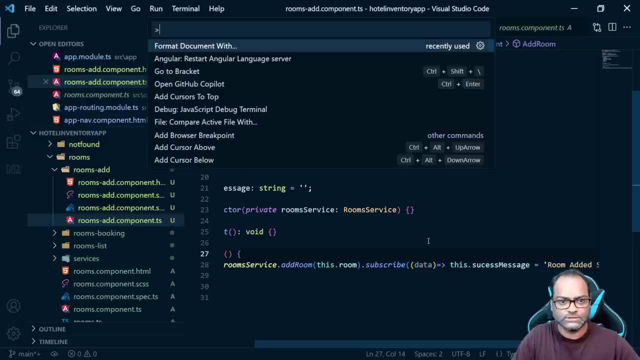 i'll say this dot. i'll say this dot message: success message is equals to: let's see what. let's see what. let's see what room edit successfully. this is what we room edit successfully. this is what we room edit successfully. this is what we needed and let me just format. 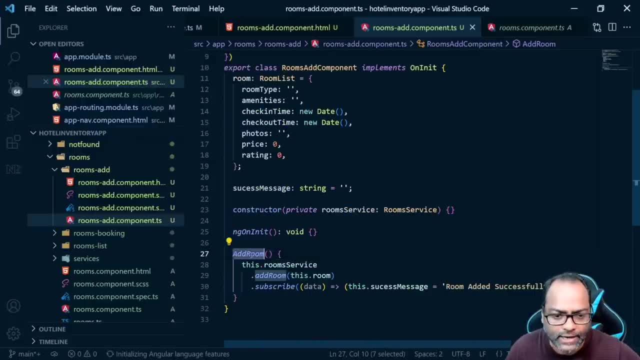 needed and let me just format needed and let me just format. so everything is visible here. so now we so everything is visible here. so now we so everything is visible here. so now we have uh add room functionality. uh, we have uh add room functionality. uh, we have uh add room functionality. uh, we injected the service, we added a success. 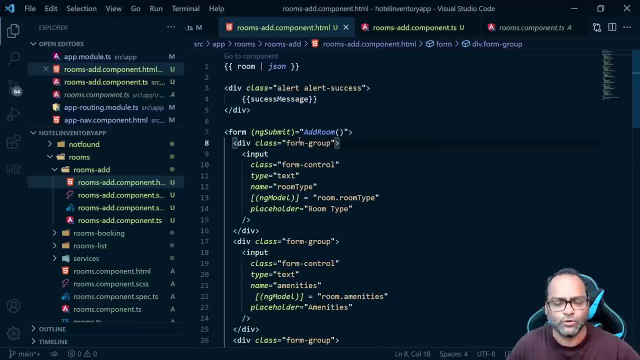 injected the service, we added a success. injected the service, we added a success message which will display in case our message, which will display in case our message, which will display in case our room is added or not, room is added or not, room is added or not. let's go ahead and 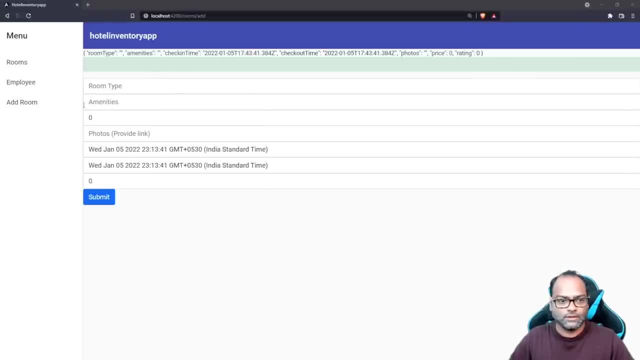 let's go ahead and let's go ahead and verify so so. so here i'll say room type is here. i'll say room type is here. i'll say room type is economy, economy, economy. amenities is: uh, we have wi-fi, uh ac, uh, ac, uh, ac. and prices, let's say, 5000 photos provide. 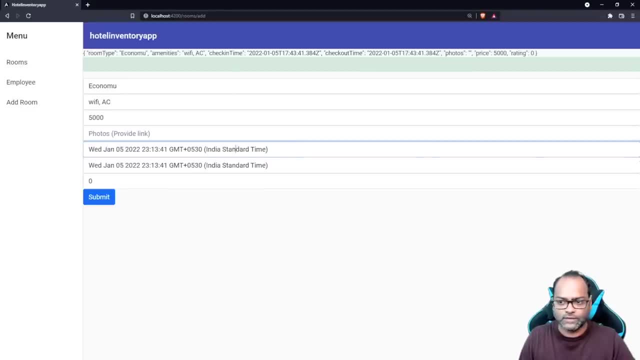 and prices. let's say 5000 photos provide and prices. let's say 5000 photos provide. link uh with. let's say link uh with. let's say link uh with. let's say: leave it right now and link uh with. let's say: leave it right now and. 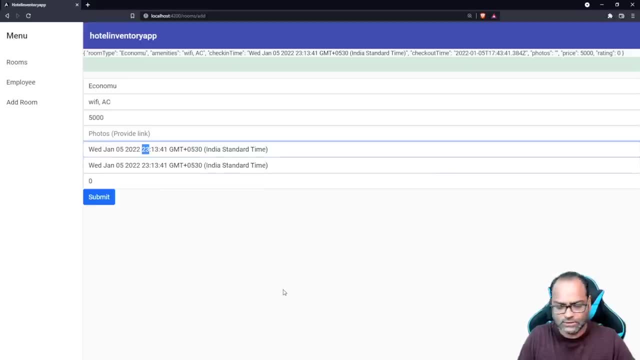 link, uh with- let's say, leave it right now, and uh, this is uh, this is uh, this is 23. let's make it 10, 23, let's make it 10, 23, let's make it 10. uh, and that's 23. uh, and that's 23. 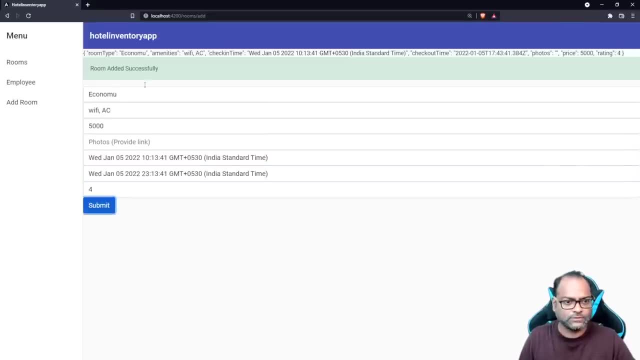 uh, and that's 23. let's provide rating. let's provide rating. let's provide rating. or or or. let's to submit and it says rooms added. let's to submit and it says rooms added. let's to submit and it says rooms added. successfully, but successfully, but. 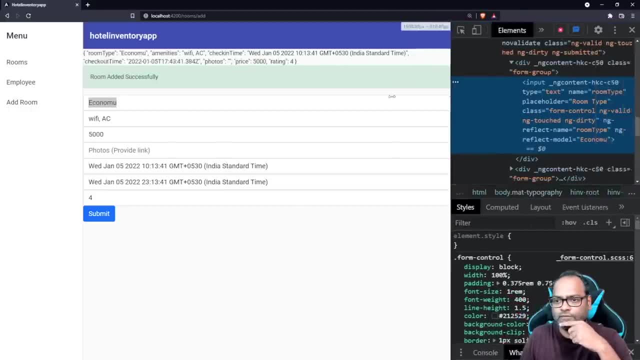 successfully. but why should we trust it right? so let's go. why should we trust it right? so let's go. why should we trust it right? so let's go ahead and ahead and ahead and verify in the console, and verify in the console, and verify in the console, and let's go to the network tab. 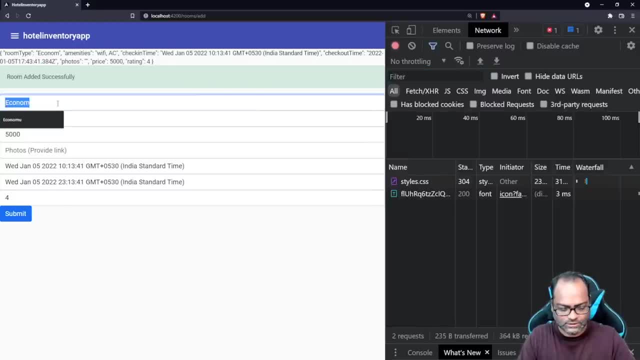 let's go to the network tab. let's go to the network tab and let's add another one right economy and let's add another one right economy and let's add another one right economy, and this is uh deluxe room, and we will say 6000, and let's click on. 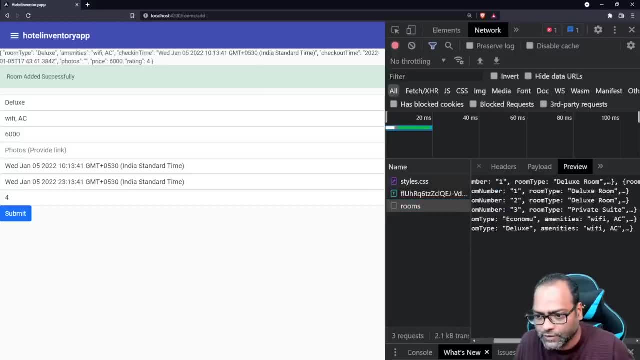 and we will say 6000 and let's click on, and we will say 6000 and let's click on submit and submit and submit and rooms is added. you can see, uh, you have rooms is added. you can see, uh, you have rooms is added. you can see, uh, you have two extra values available. room type: 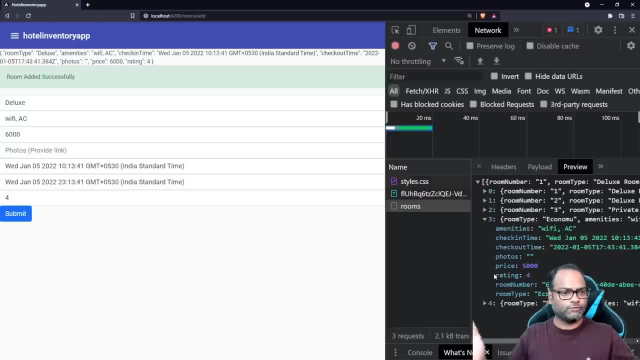 two extra values available room type. two extra values available room type. amenities and everything. amenities and everything, amenities and everything, and this is it so. what we have done is, and this is it so. what we have done is, and this is it so. what we have done is we just created our first template. 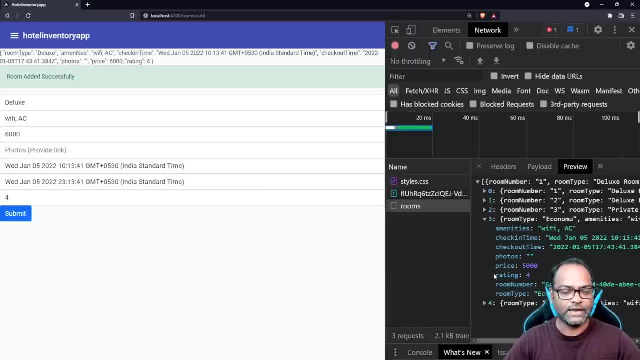 we just created our first template. we just created our first template- driven form, we driven form, we driven form, we attached. or we added the functionality attached, or we added the functionality attached, or we added the functionality to send the data to the back end: the. to send the data to the back end, the. 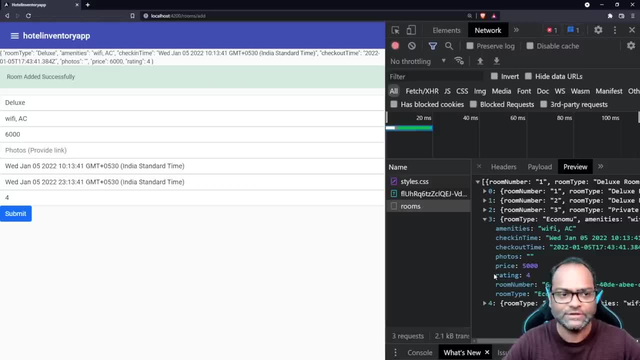 to send the data to the back end. the only thing is only thing is only thing is: the spaces are not working properly. but the spaces are not working properly. but the spaces are not working properly. but we will fix those, not an issue. we will fix those, not an issue. 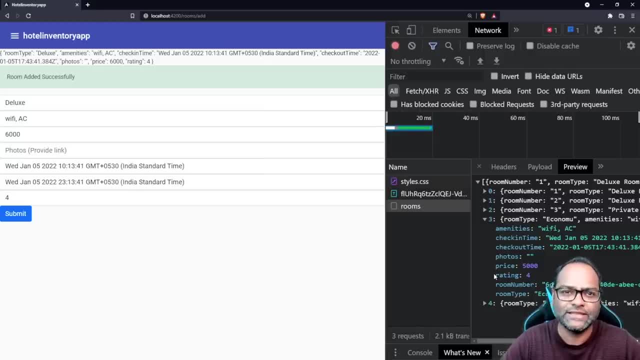 we will fix those, not an issue. and you can say that rooms added. and you can say that rooms added. and you can say that rooms added successfully- was already there successfully. was already there successfully. was already there. which doesn't look good, so we will see. which doesn't look good, so we will see. 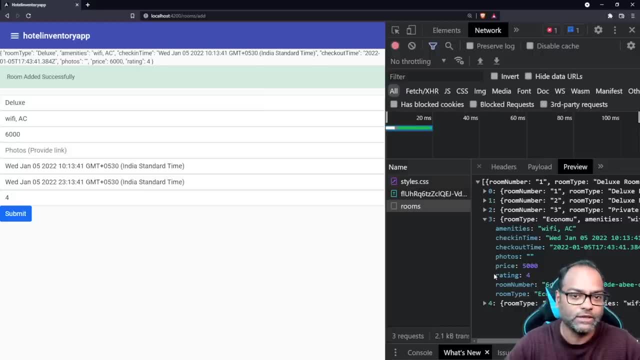 which doesn't look good. so we will see how we can actually avoid that as well, how we can actually avoid that as well, how we can actually avoid that as well. we should get it once the submit. we should get it once the submit. we should get it once the submit button is enabled or, sorry, once the 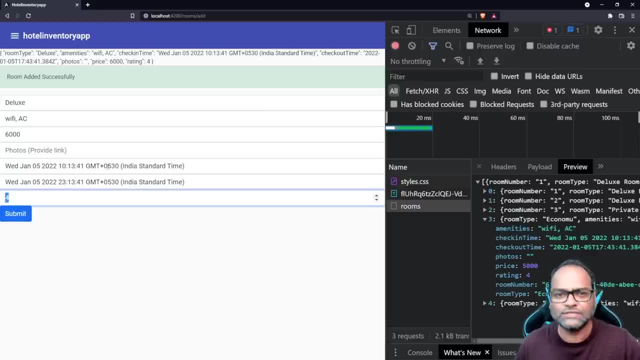 button is enabled or sorry. once the button is enabled or sorry, once the form is submitted, form is submitted. form is submitted. and also, if you notice there is no, and also if you notice there is no, and also if you notice there is no validation, validation, validation, so we can just empty, we can just enter. 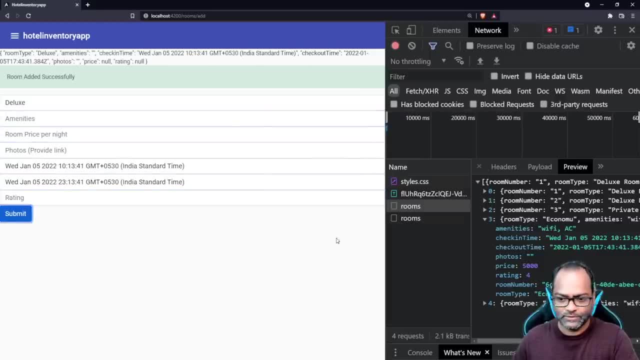 so we can just empty. we can just enter, so we can just empty. we can just enter an empty forms. i mean i can just avoid an empty forms. i mean i can just avoid an empty forms. i mean i can just avoid all the values. click on submit and. 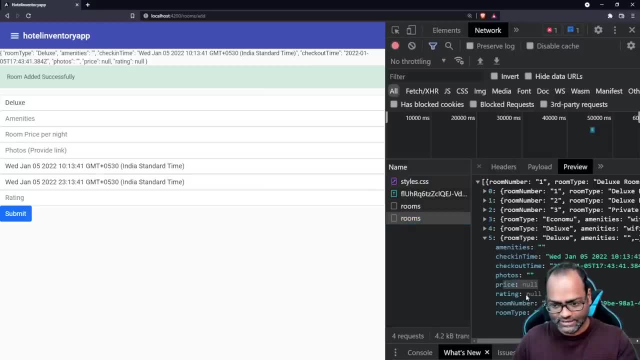 all the values. click on submit. and all the values. click on submit. and still we are able to add the room. you still we are able to add the room. you still we are able to add the room. you can see: price is null, rating is null. can see: price is null, rating is null. 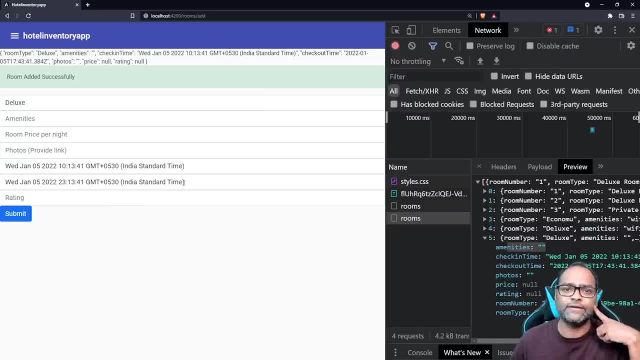 can see: price is null, rating is null and there are no amenities. so and there are no amenities, so and there are no amenities, so let's go ahead and add validation next. let's go ahead and add validation next. let's go ahead and add validation next time, then we will see. 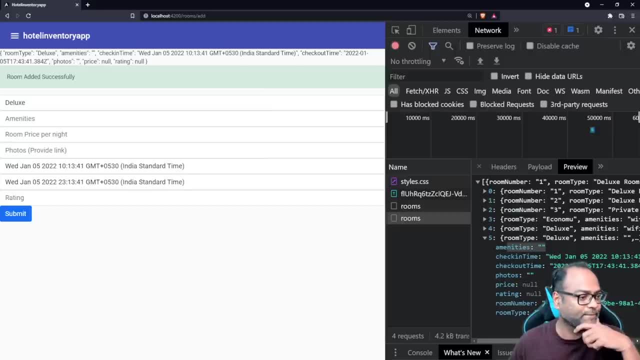 time, then we will see time. then we will see some more functionality related to our, some more functionality related to our, some more functionality related to our template driven forms. let's go ahead and add some validations. let's go ahead and add some validations. let's go ahead and add some validations to this form, because we haven't done. 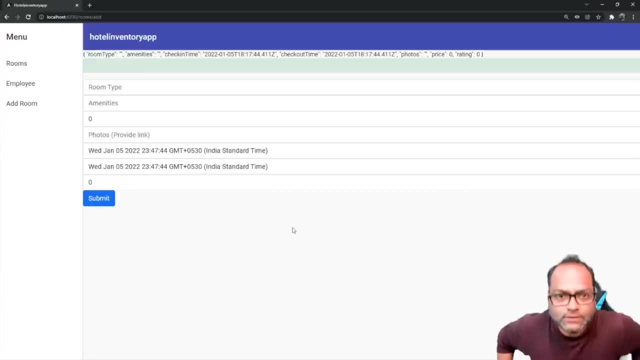 to this form because we haven't done to this form, because we haven't done that right and we can just that right and we can just that right and we can just, we can just submit a blank form as of now. we can just submit a blank form as of now. 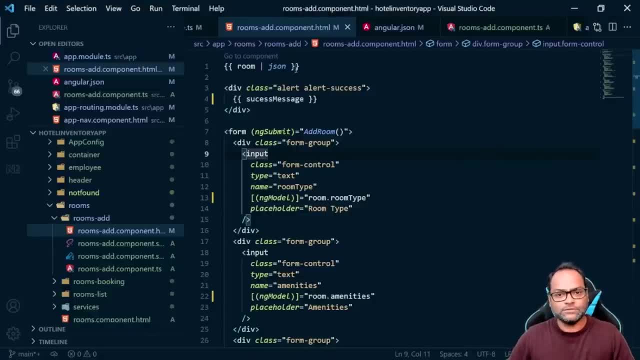 we can just submit a blank form as of now to add validation, to add validation. to add validation in template driven forms. we have to use in template driven forms. we have to use in template driven forms. we have to use the html5 validations. so, in case you are, 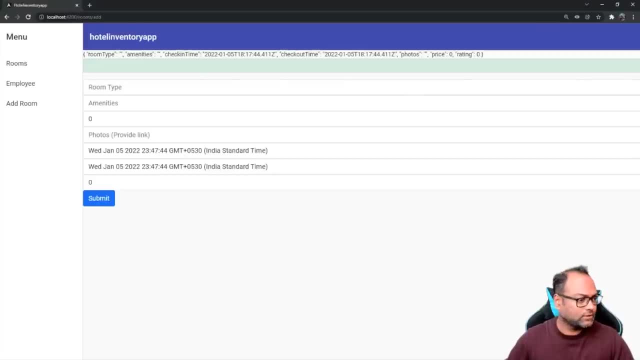 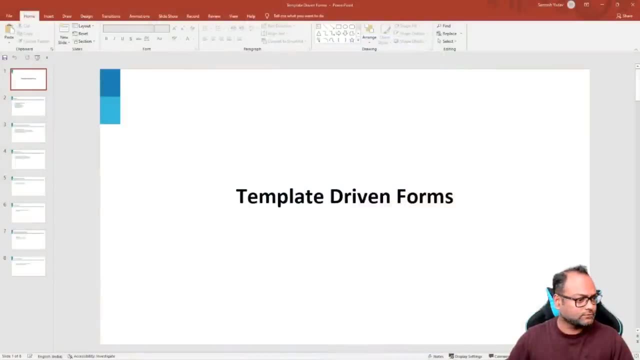 the html5 validations. so, in case you are the html5 validations. so, in case you are not aware of what html5 validations, are not aware of what html5 validations, are not aware of what html5 validations are, let me just, let me just, let me just go back to 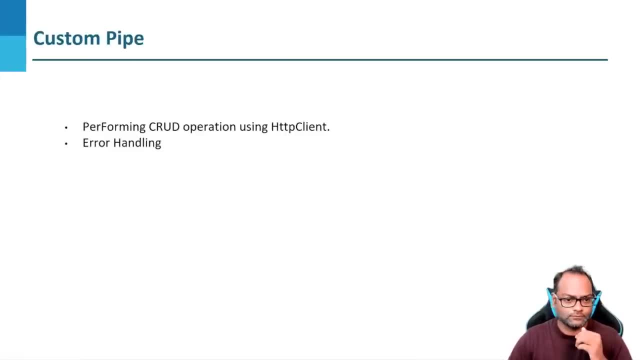 go back, to go back to: yeah, so, uh, we, as you said, we will be. yeah, so, uh, we, as you said, we will be. yeah, so, uh, we, as you said, we will be using html for using html, for using html for five forms and, uh, sorry, html5 validators. 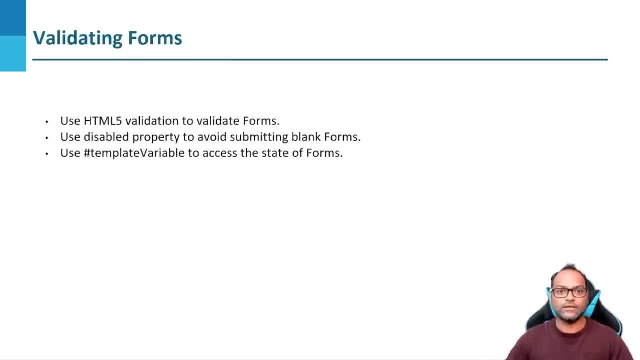 five forms and, uh sorry, html5 validators. five forms and, uh sorry, html5 validators. so there are multiple validators which. so there are multiple validators which. so there are multiple validators which exist. so let's go ahead and exist. so let's go ahead and exist. so let's go ahead and uh see them. 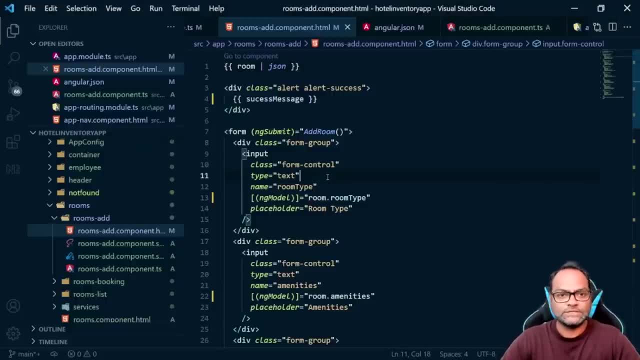 first. so the first time i think first. so the first time i think first. so the first time i think uh first time. i think uh first time, i think uh first time. i think most of the time you will be using this, most of the time you will be using this. most of the time, you will be using this validator, which is known as required. so, validator which is known as required, so validator which is known as required. so let's go ahead and see, uh, how we can add. let's go ahead and see, uh, how we can add. 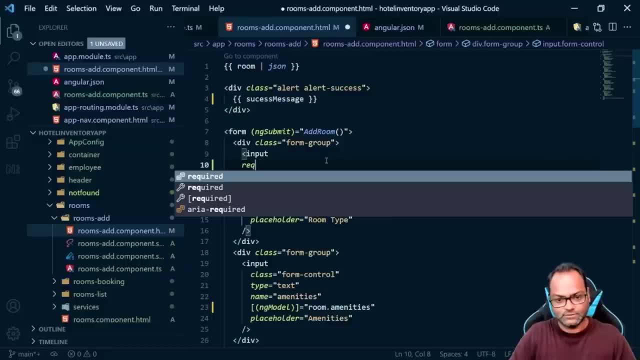 let's go ahead and see, uh, how we can add that. so to add a required validator, you that. so to add a required validator, you that. so to add a required validator, you have to just say required. have to just say required, have to just say required. that's it. yeah, that's, uh, that's. 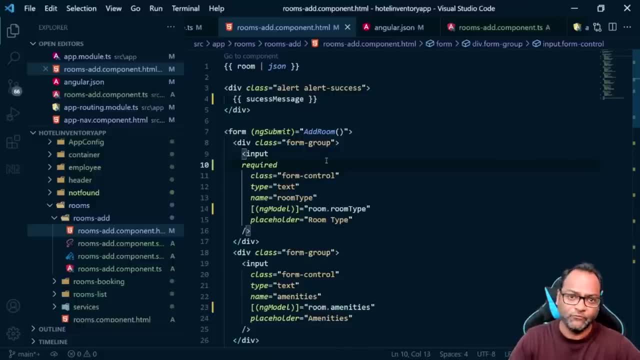 that's it. yeah, that's uh. that's that's it. yeah, that's uh, that's. you are done so. you have added a. you are done so. you have added a. you are done so. you have added a required validator. and now this required validator, and now this: 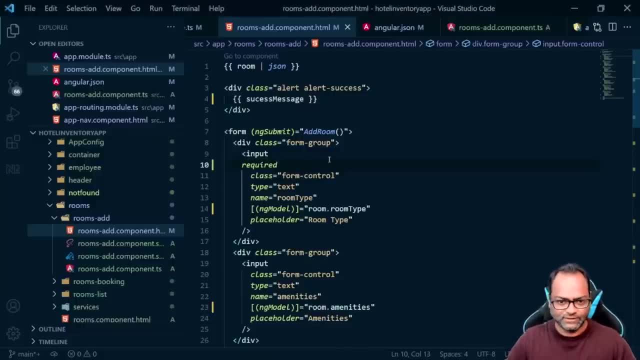 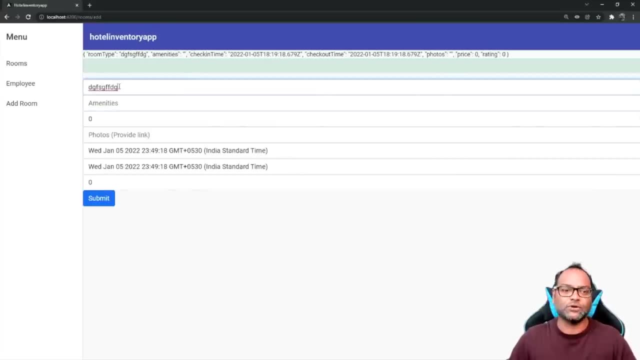 required validator, and now this field becomes required, but field becomes required, but field becomes required. but let's go ahead and verify: does it look like it is required? does it look like it is required? does it look like it is required? of course, no, because we have to add some. 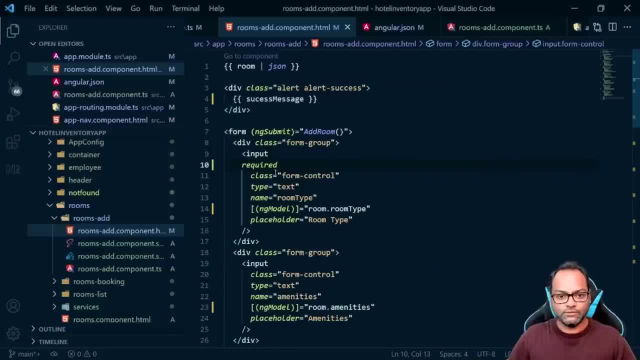 of course no, because we have to add some. of course no, because we have to add some extra checks. we'll talk about it. extra checks, we'll talk about it. extra checks, we'll talk about it. let's go back to the code. let's add the. let's go back to the code. let's add the. 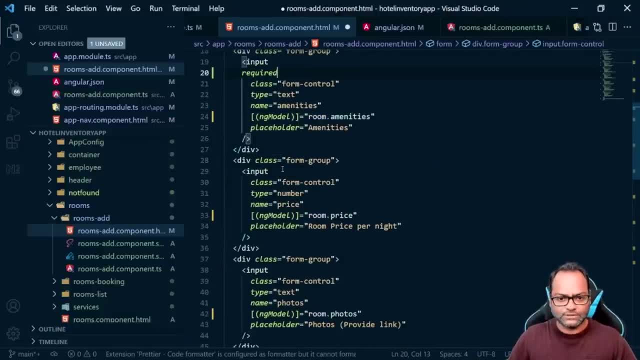 let's go back to the code. let's add the fields right now. so we'll say, okay, fields right now. so we'll say okay, fields right now. so we'll say, okay, right now, required. this is required. this right now required. this is required. this right now required. this is required. this is also required. 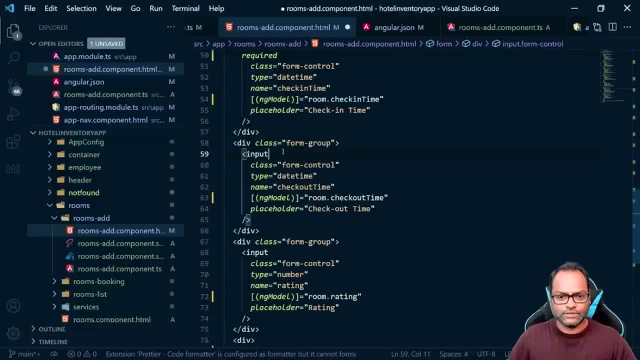 is also required. is also required. this is required. this is required. this is required, right so, all the form fields are required, right so, all the form fields are required, right so, all the form fields are required right now. but we can still go ahead and submit the. but we can still go ahead and submit the. 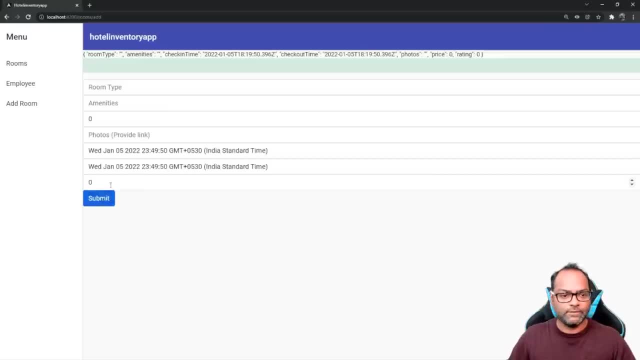 but we can still go ahead and submit the button now. button now. button now. let's see how we can actually uh. i mean, let's see how we can actually uh. i mean, let's see how we can actually uh. i mean, we can still go ahead and see the submit. 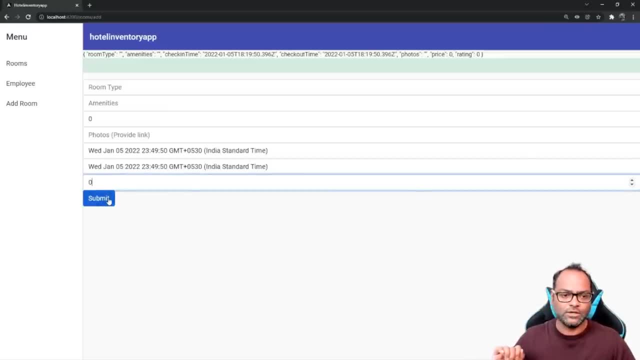 we can still go ahead and see the submit. we can still go ahead and see the submit: button, button, button. so let's see how we can actually. so let's see how we can actually. so let's see how we can actually disable this control. disable this control. 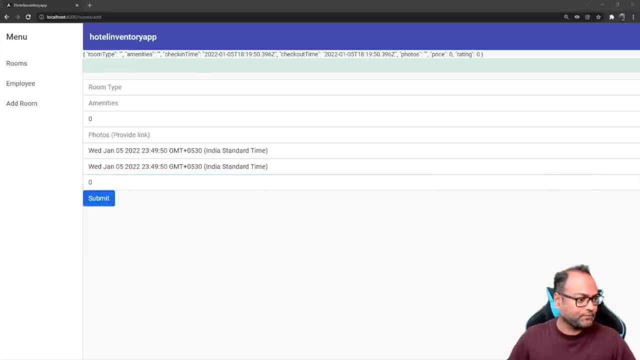 disable this control until unless we have received all the. until, unless we have received all the. until, unless we have received all the values and valid values, values and valid values, values and valid values. let's go back so, uh, to actually get. let's go back so, uh, to actually get. 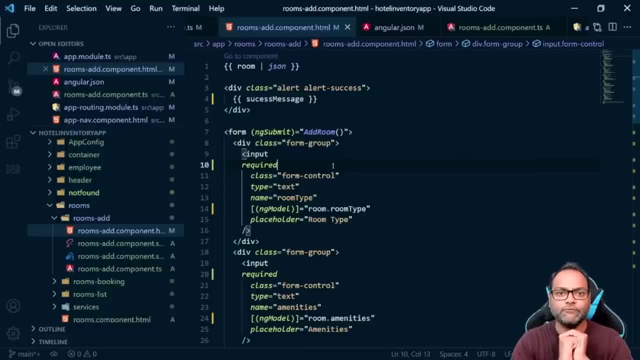 let's go back so, uh, to actually get the status, the status, the status of my form, whether this form is valid or of my form, whether this form is valid or of my form, whether this form is valid or not. we need to get an instance of this. 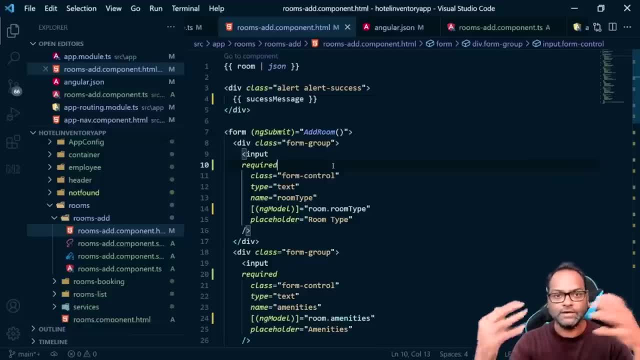 not, we need to get an instance of this, not we need to get an instance of this form. how we can do that form, how we can do that form, how we can do that right. i mean we have talked about right. i mean we have talked about right. i mean we have talked about classes. to create a instance of a class. 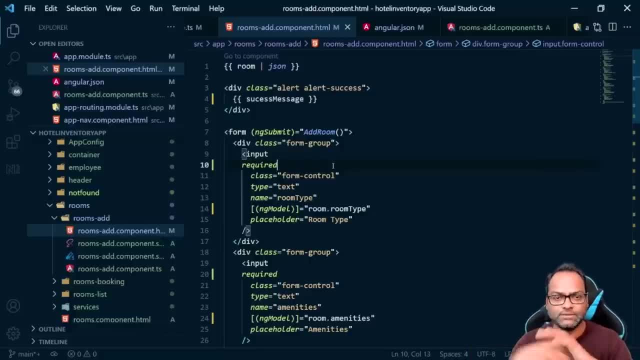 classes to create a instance of a class. classes to create a instance of a class. we do, we do, we do. object equals to new, and then whatever object equals to new, and then whatever object equals to new, and then whatever class name is. class name is, class name is. so we said hash and some name, and then 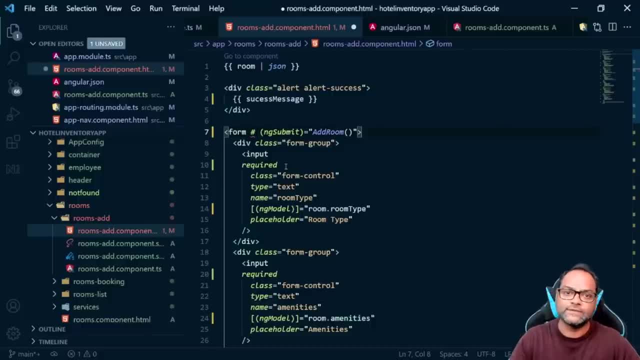 so we said hash and some name. and then so we said hash and some name, and then equals to equals to equals to a hash, some name, and then it gives you the a hash, some name, and then it gives you the a hash, some name, and then it gives you the instance of that particular. 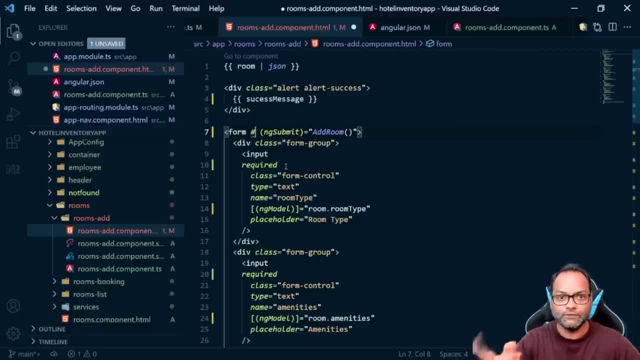 instance of that particular instance of that particular, uh particular html control right. we, we uh particular html control right. we we uh particular html control right. we we discussed it for, discussed it for, discussed it for div. so here also we can actually use div. so here also we can actually use. 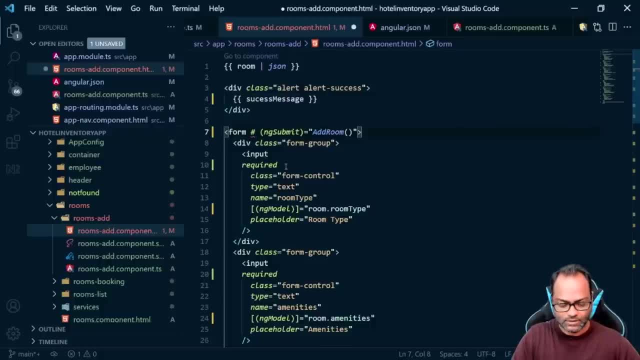 div. so here also we can actually use this way, so i can say this is a this way, so i can say this is a this way, so i can say this is a rooms form, rooms, form, rooms. form is equals to you have to say ng form is equals to you have to say ng form. 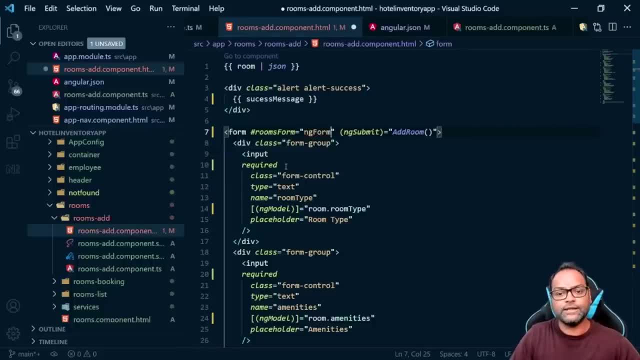 is equals to, you have to say ng form, remember this ng form, remember this ng form, remember this ng form. and now you will, you get an instance of, and now you will, you get an instance of, and now you will, you get an instance of this form, this form. 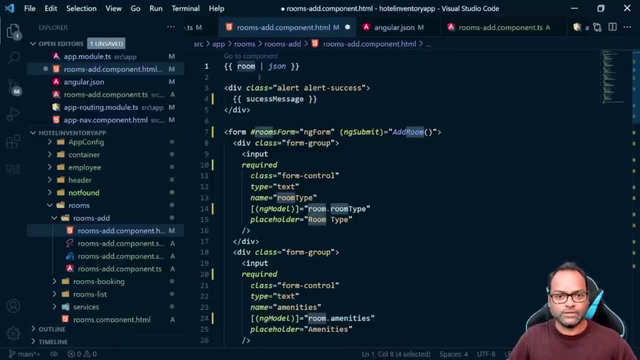 this form to yourself, now how we can verify so to yourself, now how we can verify so to yourself, now how we can verify so let's uh avoid, let's remove this and let's uh avoid. let's remove this and let's uh avoid. let's remove this and use rooms form here. 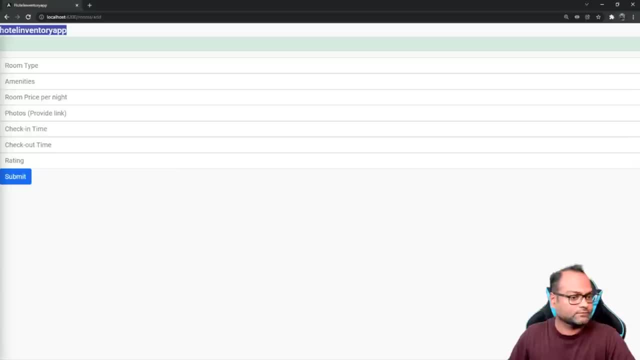 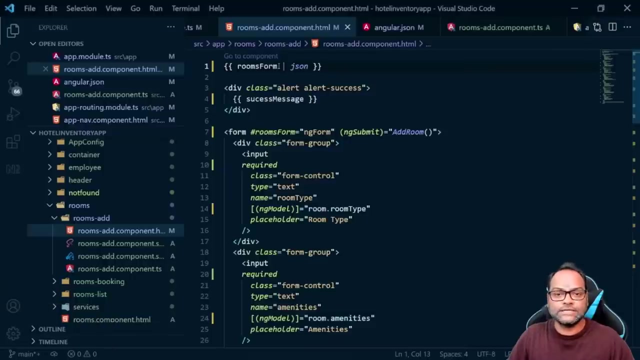 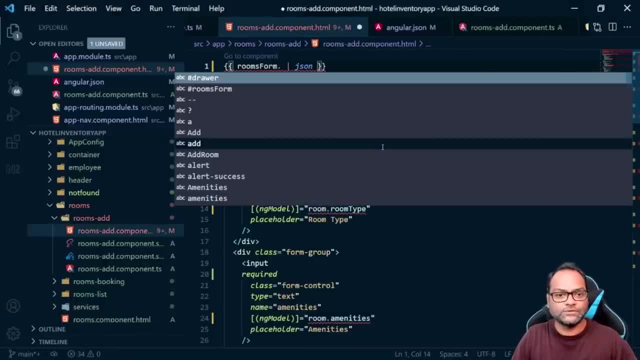 because, uh, this json has a lot of, because, uh, this json has a lot of properties. so, right now, what the properties? so, right now, what the properties? so, right now, what the property which we need is rooms form uh. property which we need is rooms form uh, property which we need is rooms form, uh, we need. 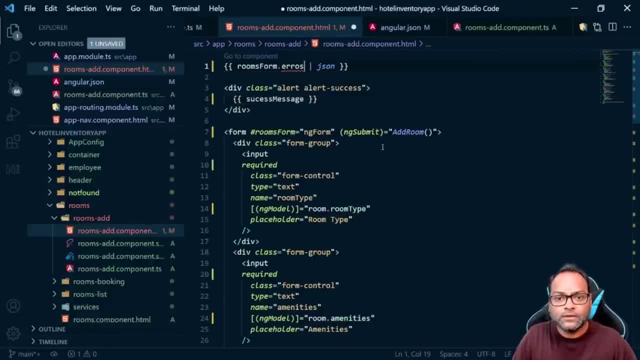 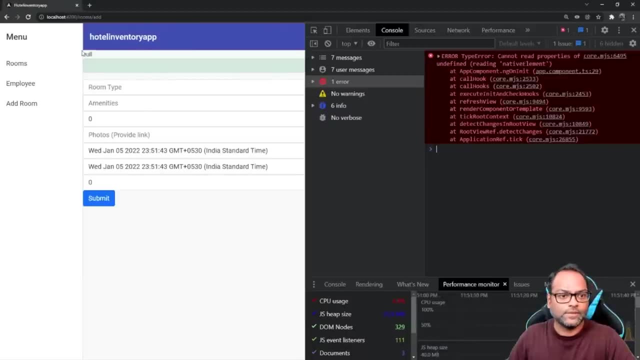 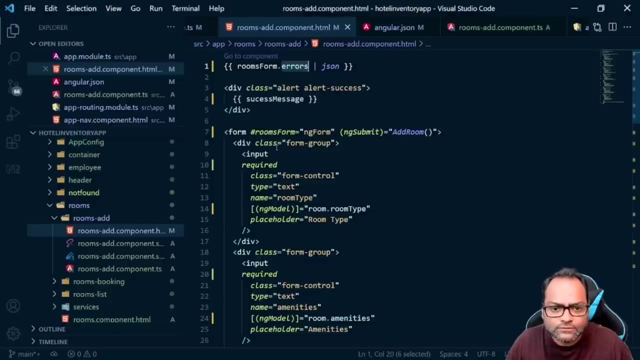 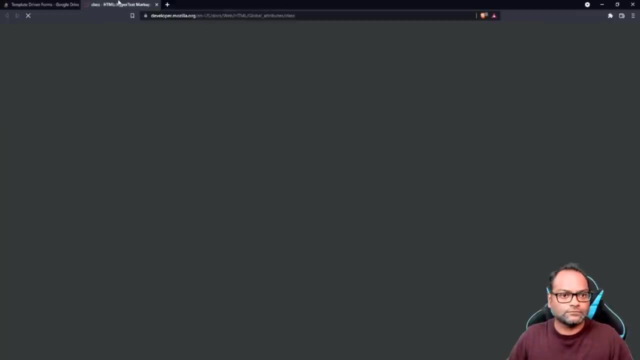 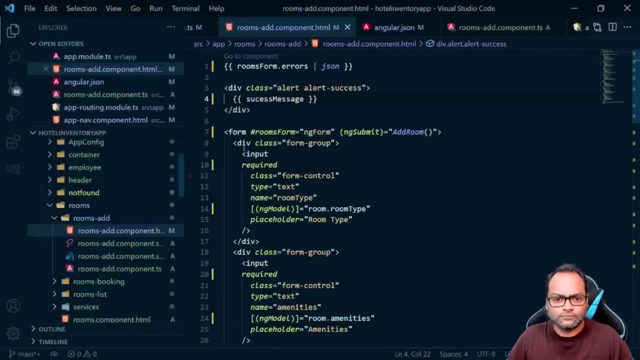 we need, we need errors. double rs. yeah, we need rs property. let's double rs. yeah, we need rs property. let's double rs. yeah, we need rs property. let's go ahead and see. so uh, it says null. why so so? so, so, uh, it says null, why so so? 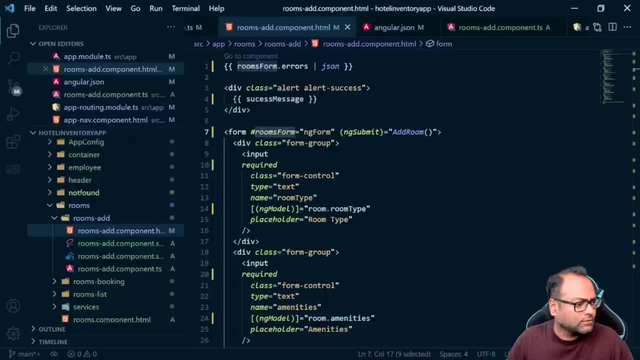 so we have tombs form, we have tombs form, we have tombs form. okay. so, uh, the property which we need is okay. so, uh, the property which we need is okay. so, uh, the property which we need is valid, so it has two properties. uh, all the. 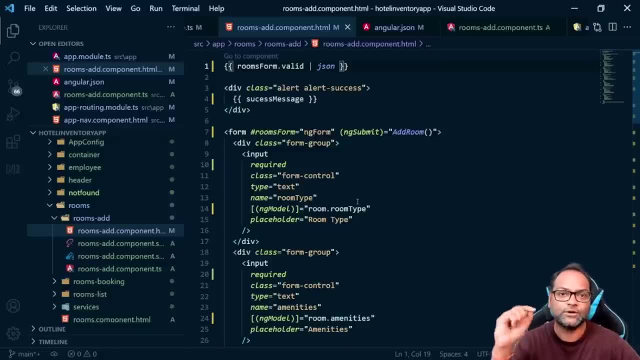 valid, so it has two properties. uh, all the valid, so it has two properties. uh, all the forms, all html forms, has this, all this forms, all html forms has this, all this forms, all html forms has this, all this property. so it's not like it is available. 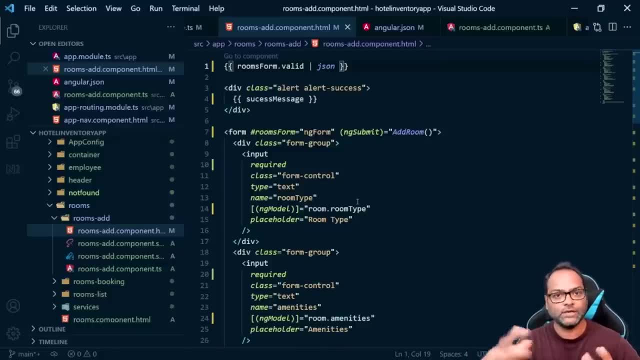 property, so it's not like it is available property. so it's not like it is available only for angular. no, it's not. it is uh only for angular? no, it's not. it is uh only for angular? no, it's not. it is uh available in normal html as well. you can. 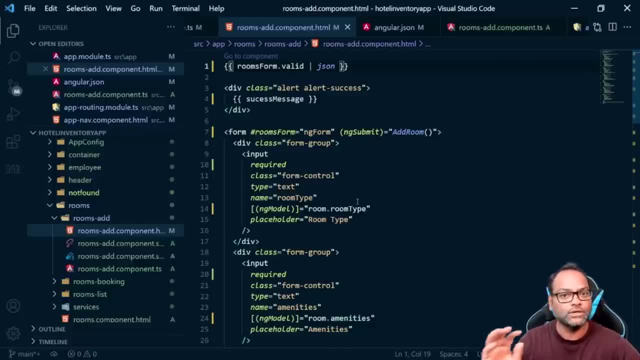 available in normal html as well. you can available in normal html as well. you can actually access these properties via. actually access these properties via. actually access these properties via javascript, in case you want to, if you javascript, in case you want to, if you javascript in case you want to, if you are writing a normal javascript or 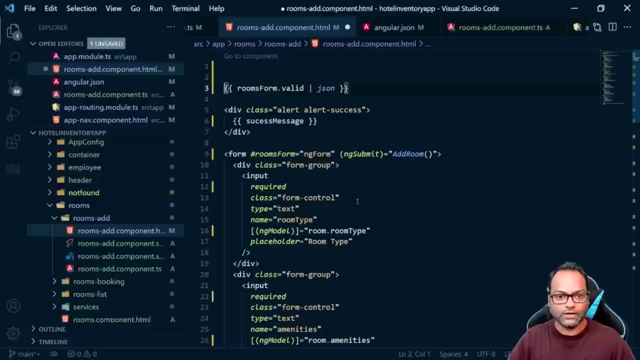 are writing a normal javascript or are writing a normal javascript or typescript code. so let's talk about all typescript code. so let's talk about all typescript code. so let's talk about all these properties which we are going to, these properties which we are going to. 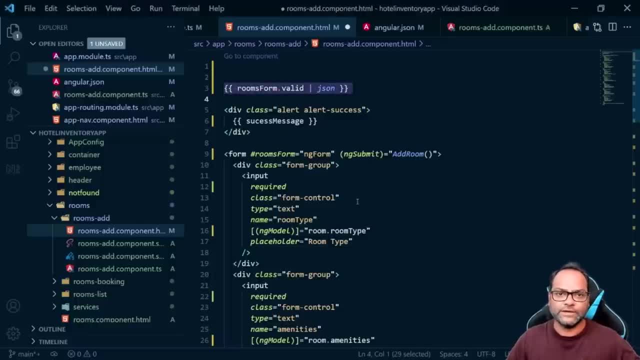 these properties which we are going to see, so see, so see, so valid, will tell us whether this form is valid. will tell us whether this form is valid. will tell us whether this form is valid or not. let's verify valid or not. let's verify valid or not. let's verify so. it says false. so the current form is. 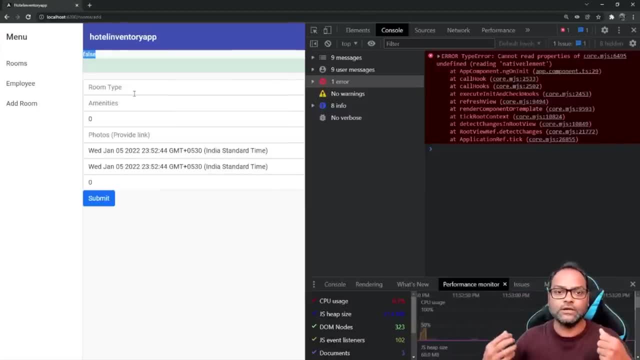 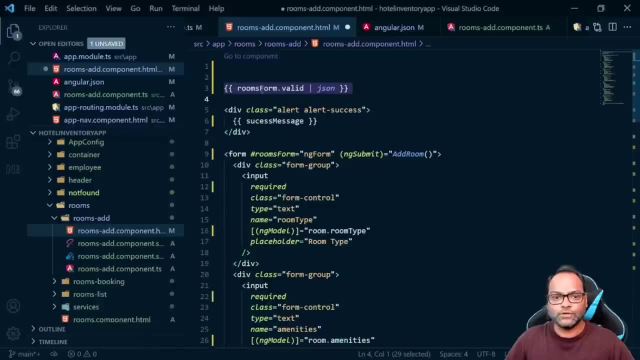 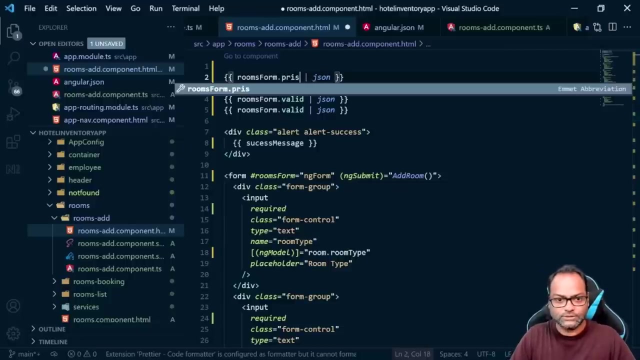 so it says false. so the current form is. so it says false. so the current form is not valid. not valid, not valid, we'll replace. so we are going to talk, we'll replace. so we are going to talk, we'll replace. so we are going to talk about something known as pristine. 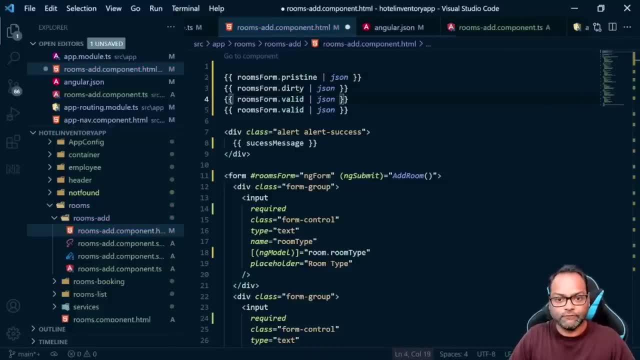 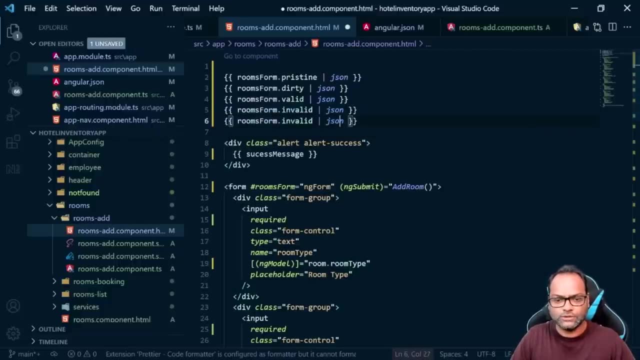 then we'll talk about something known, then we'll talk about something known, then we'll talk about something known as dirty, as dirty, as dirty, valid, invalid, valid, invalid, valid, invalid. and we also have something known as, and we also have something known as, and we also have something known as value. 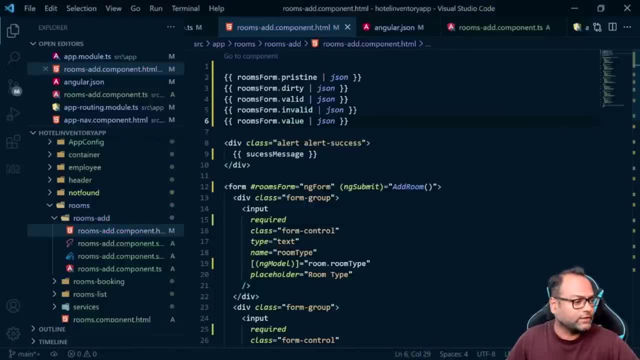 value, not values. let's see, let's see what value not values. let's see, let's see what value not values. let's see, let's see what we get here. so we have true, false, false, true, and so we have true, false, false, true, and so we have true, false, false, true, and then 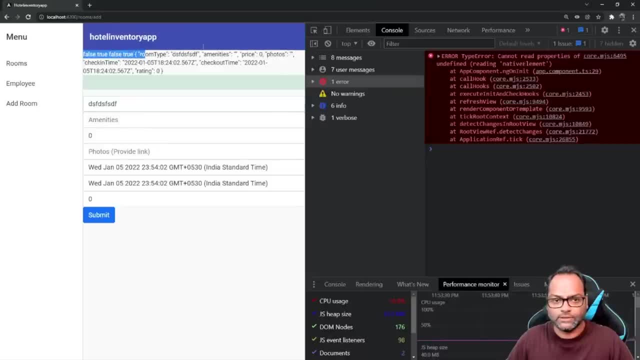 then, then this is: this is: this: is your forms value right? whatever you, your forms value right? whatever you, your forms value right. whatever you enter here will be available here. enter here will be available here. enter here will be available here. you don't have to necessarily, uh, take the. 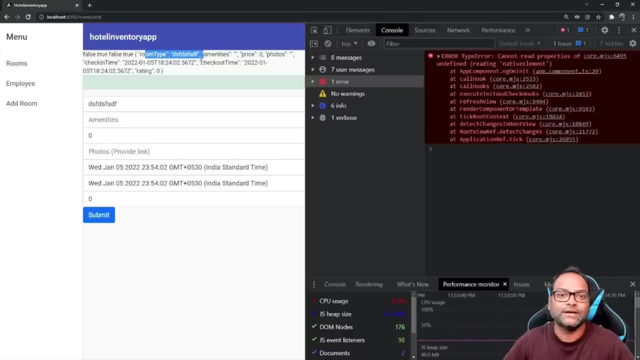 you don't have to necessarily uh take the. you don't have to necessarily uh take the value from form dot value. you can also value from form dot value. you can also value from form dot value. you can also get it from your, get it from your, get it from your uh. of course, the model which you have. 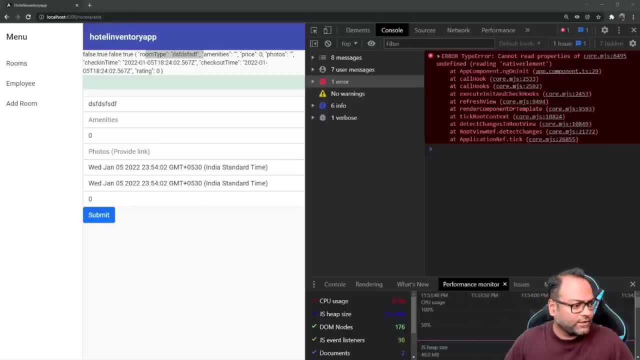 uh, of course, the model which you have. uh, of course, the model which you have created, created, created. so, here, uh, let's go ahead and see what. so here, uh, let's go ahead and see what. so here, uh, let's go ahead and see what these values are. false, true, false, true. 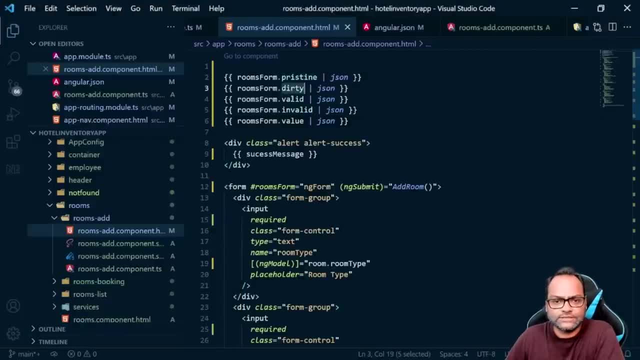 these values are false, true, false, true. these values are false, true, true, right, let's see. so this is pristine, this right, let's see. so this is pristine, this right, let's see. so this is pristine. this is dirty, this is valid, and this is is dirty, this is valid and this is. 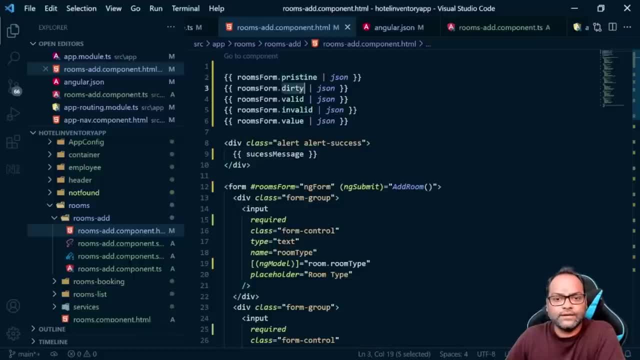 is dirty, this is valid and this is invalid. so what are these values so invalid? so what are these values so invalid? so what are these values? so? pristine and dirty are real, uh, in good pristine and dirty are real, uh, in good pristine and dirty are real, uh, in good use cases. i'll talk about it, let's talk. 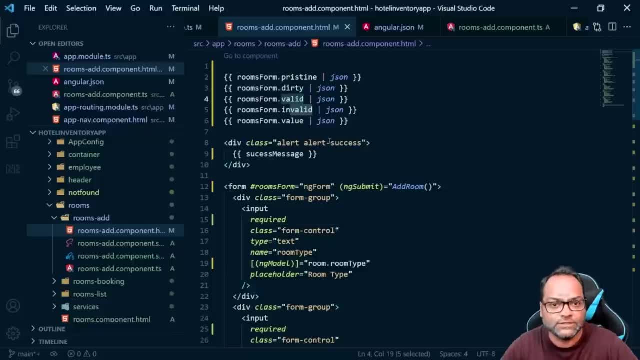 use cases. i'll talk about it. let's talk use cases. i'll talk about it. let's talk about valid and invalid right. so they about valid and invalid right. so they about valid and invalid right. so they are like opposite of each other. so are like opposite of each other. so 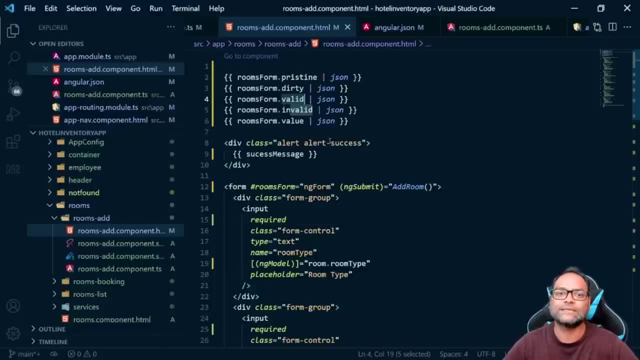 are like opposite of each other. so if your any of your, if your any of your, if your any of your, all the form control uh becomes error. all the form control uh becomes error. all the form control uh becomes error. free, it means they don't uh. free, it means they don't uh. 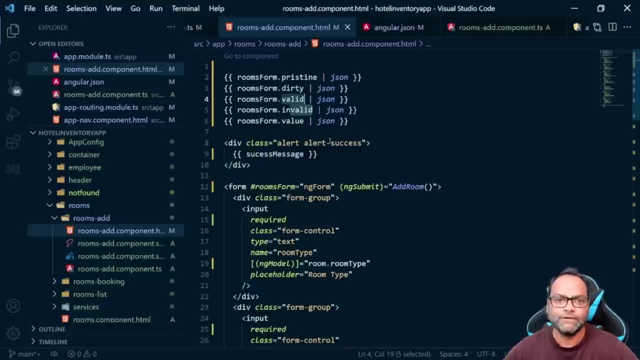 free. it means they don't- uh, don't break any validation rule which you don't break any validation rule which you don't break any validation rule which you have provided. it means they are valid. have provided it means they are valid. have provided. it means they are valid, which will be true and invalid will. 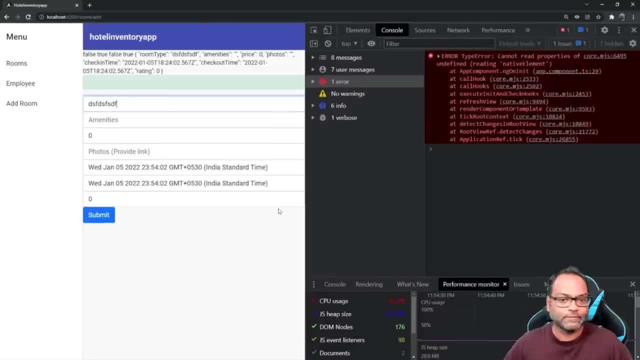 which will be true and invalid will, which will be true and invalid will become false. so here, if you see become false. so here, if you see become false. so here, if you see currently, currently, currently, if you see currently, it says uh. if you see currently it says uh. 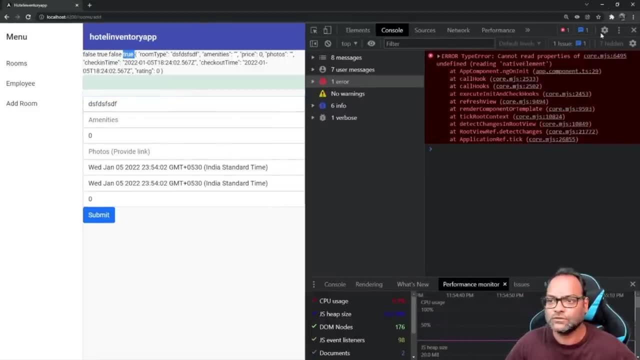 if you see, currently it says: uh, valid is false and invalid is true, which valid is false and invalid is true, which valid is false and invalid is true, which is true, right, so let's see how we can. is true, right, so let's see how we can. 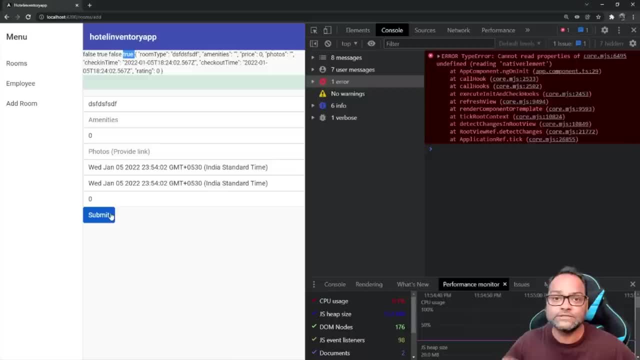 is true, right, so let's see how we can actually disable this first, actually disable this first. actually disable this first. let's you uh handle this use case. where let's you uh handle this use case? where let's you uh handle this use case where how we can disable this particular. 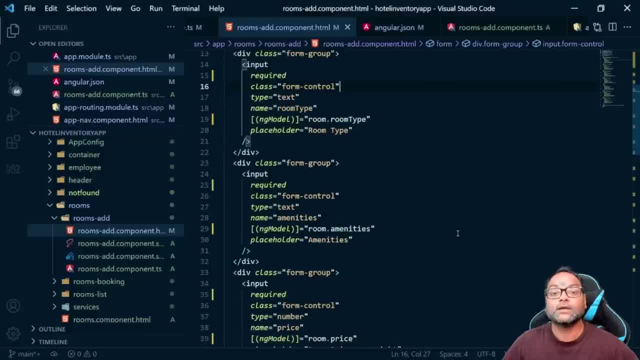 how we can disable this particular, how we can disable this particular submit button. before i go ahead and do that, let me tell, before i go ahead and do that, let me tell, before i go ahead and do that, let me tell you one thing very clear. you one thing very clear. 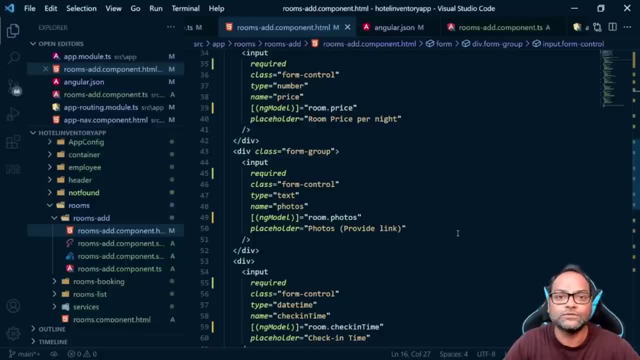 you one thing very clear: in case you have some validations, don't. in case you have some validations, don't. in case you have some validations, don't just add those validations at your. just add those validations at your. just add those validations at your front end. your back end should also have. 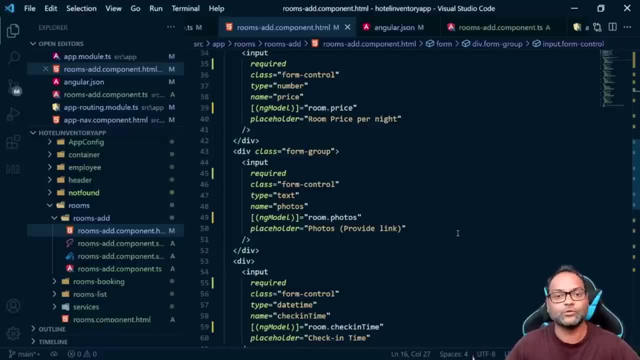 front end. your back end should also have front end. your back end should also have those same validation. because what you, those same validation. because what you, those same validation. because what you are going to do is end of the day there are going to do is end of the day there. 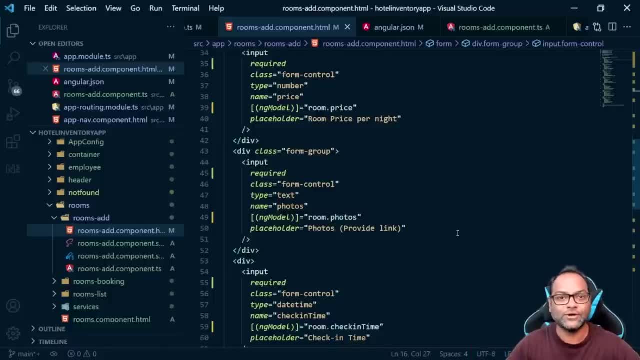 are going to do is, end of the day, there will be an api call will be an api call will be an api call and if your someone figures out how to, and if your someone figures out how to, and if your someone figures out how to make your api calls and without passing, 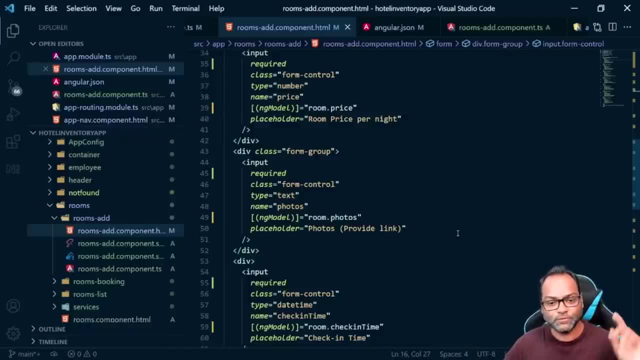 make your api calls and without passing. make your api calls and without passing the data. if you the data, if you the data, if you you'll be able to break your system. so you'll be able to break your system. so you'll be able to break your system. so make sure that you add validation at 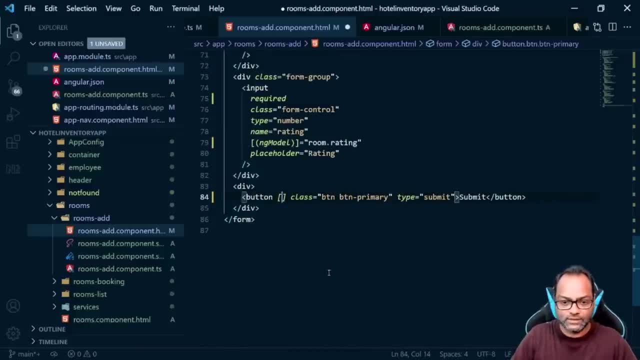 make sure that you add validation at. make sure that you add validation at both the places, not only at front end. both the places, not only at front end. both the places, not only at front end. so here you can, we can use a property. so here you can, we can use a property. 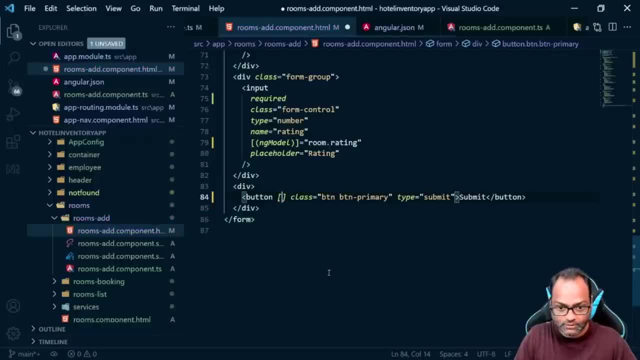 so here you can, we can use a property called invalid. we'll be using disabled and uh, we'll say we'll be using disabled and uh, we'll say we'll be using disabled and uh, we'll say rooms form dot, rooms form dot, rooms form dot. so we want it to be disabled, in case. 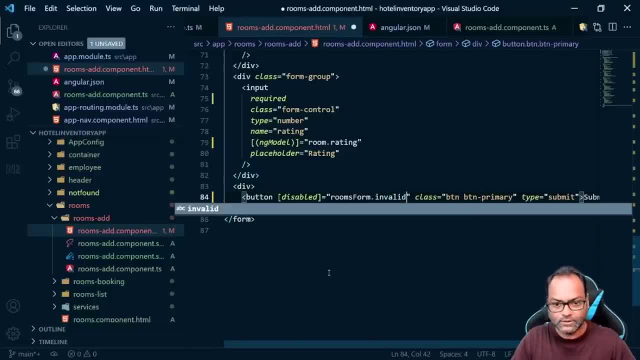 so we want it to be disabled in case. so we want it to be disabled in case. our form is invalid. so let's say our form is invalid. so let's say our form is invalid. so let's say so it should be disabled in case. our form. 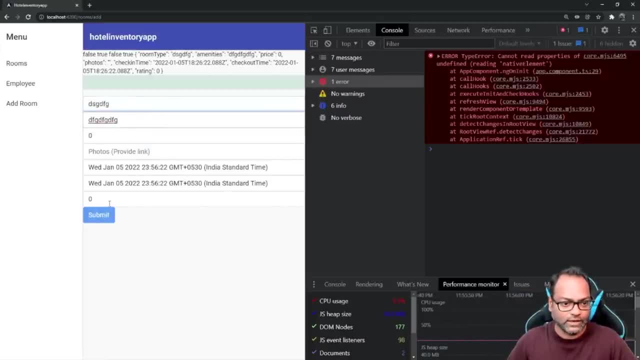 so it should be disabled in case our form is invalid. so let's enter all. the is invalid, so let's enter all. the is invalid, so let's enter all the values, values, values, and let's see. and now our form becomes valid, right you? and let's see. 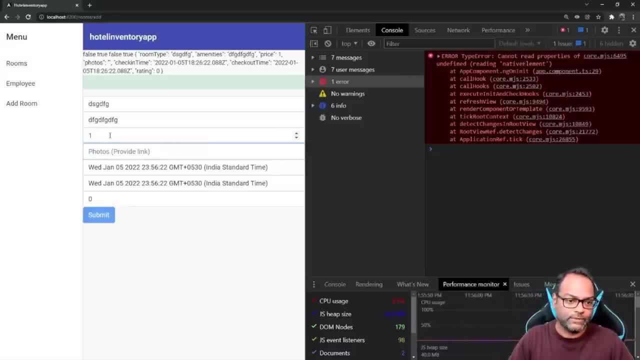 and now our form becomes valid. right, you can see this. so if i remove, can see this. so if i remove, can see this. so if i remove this value, it means my form becomes this value. it means my form becomes this value, it means my form becomes invalid again. so submit: become the. 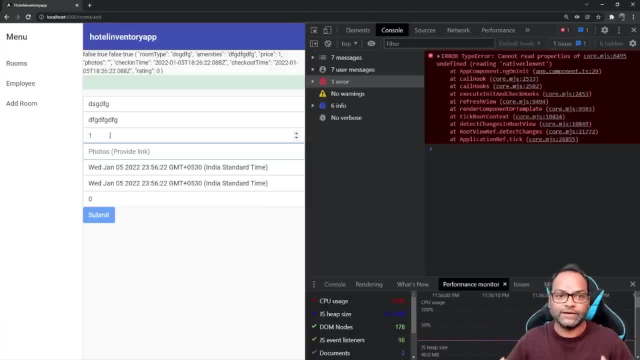 invalid again. so submit become the invalid again. so submit become the submit button becomes disabled. so this is submit button becomes disabled. so this is submit button becomes disabled. so this is how the required validator works and how the required validator works and how the required validator works, and these are the values: uh, the uh, these. 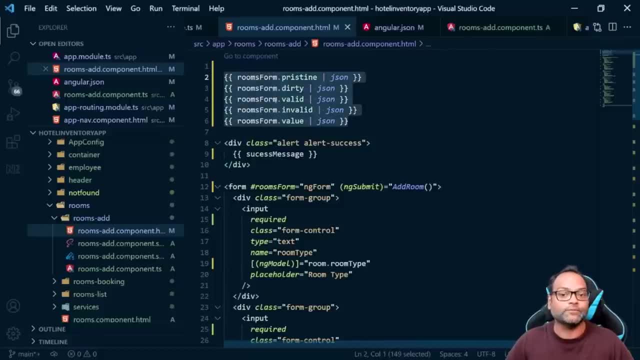 these are the values uh the uh these. these are the values uh the uh these. these are the properties which you can. these are the properties which you can. these are the properties which you can access by using this particular form. so, access by using this particular form. so. 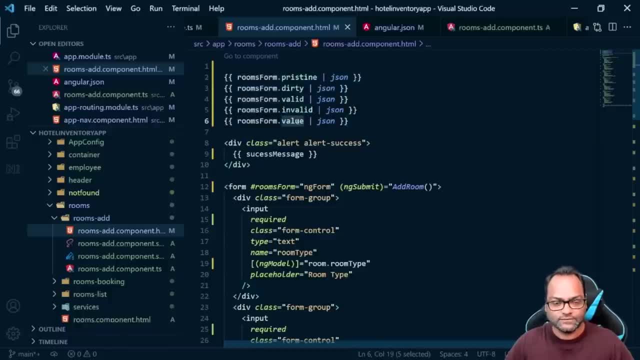 access by using this particular form. so pristine dirty invalid value, pristine dirty invalid value. pristine dirty invalid value, and uh value as well. so, and uh value as well. so, and uh value as well. so now, here also, let's do uh check. so i'll. now, here also, let's do uh check. so i'll. 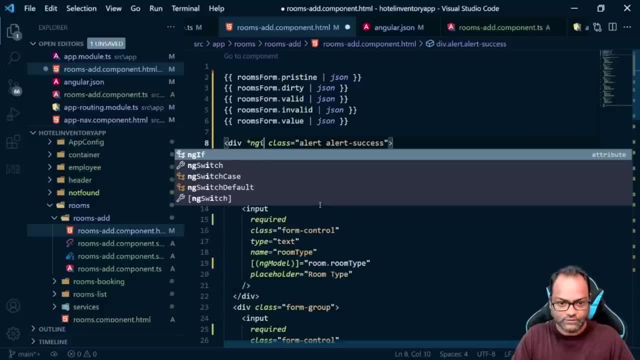 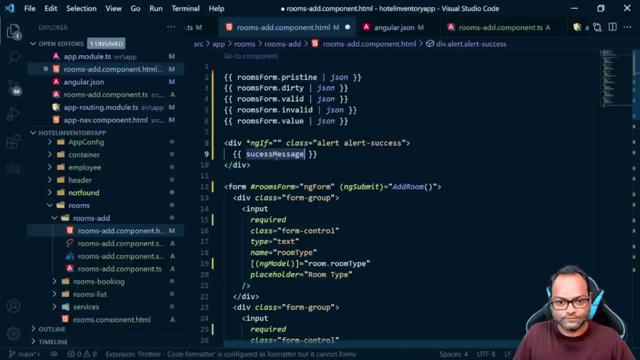 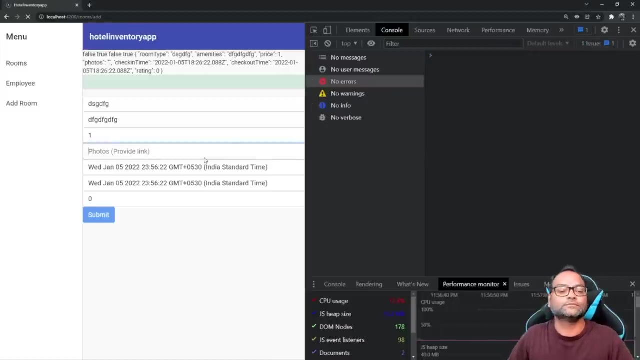 now here also let's do uh check. so i'll say this, say this, say this: start ng, if start ng, if start ng, if is equals to, we can say success message is not equals to blank, is not equals to blank. and let's see now, and let's see now. 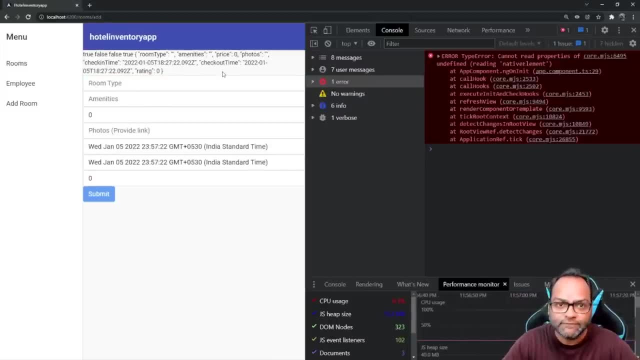 and let's see now. so this, so this, so this: the success bar should be only available. the success bar should be only available. the success bar should be only available after the submit button is clicked. and after the submit button is clicked. and after the submit button is clicked, and in case we have some message otherwise, 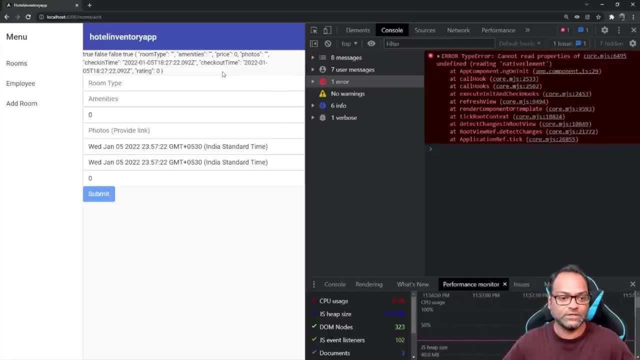 in case we have some message otherwise. in case we have some message otherwise, it won't be. it won't be, it won't be enabled, or it won't be displayed on the enabled, or it won't be displayed on the enabled or it won't be displayed on the page. so now, what we have done is we have page. so now what we have done is we have page. so now what we have done is we have taken care of two cases which we taken care of, two cases which we taken care of, two cases which we discussed about now let's go ahead and discussed about. now let's go ahead and 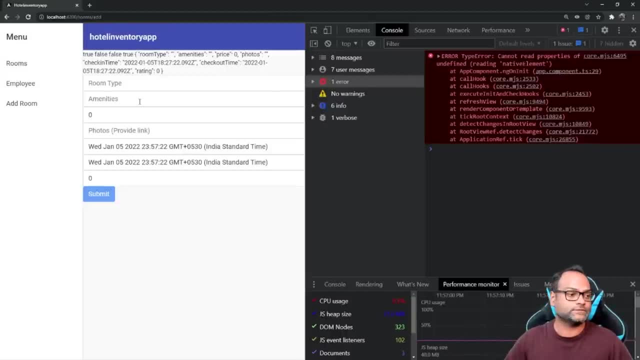 discussed about. now. let's go ahead and add more, add more, add more validators. the next validator which we are going to, the next validator which we are going to, the next validator which we are going to talk about is: uh, we'll see min and talk about is: uh, we'll see min. and. 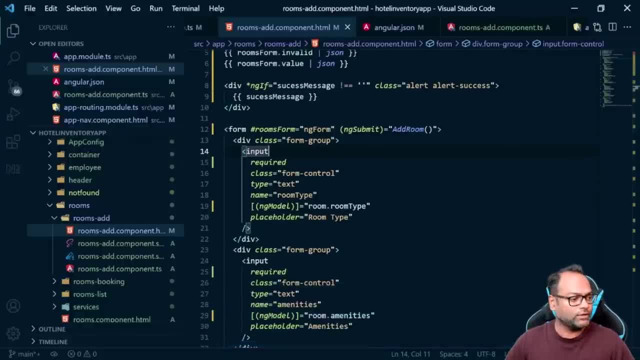 talk about is, uh, we'll see min and min length and max length. so min length and max length. so min length and max length. so what? what? what is the use cases for me length and max? is the use cases for me length and max? is the use cases for me length and max? and so in case, let's say you want, 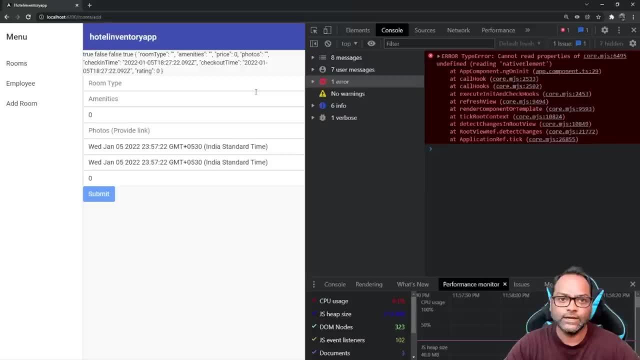 and so in case let's say: you want. and so in case let's say: you want amenities right. so, for example, let's take amenities right. so, for example, let's take amenities right. so, for example, let's take, let's, let's go ahead and do that. 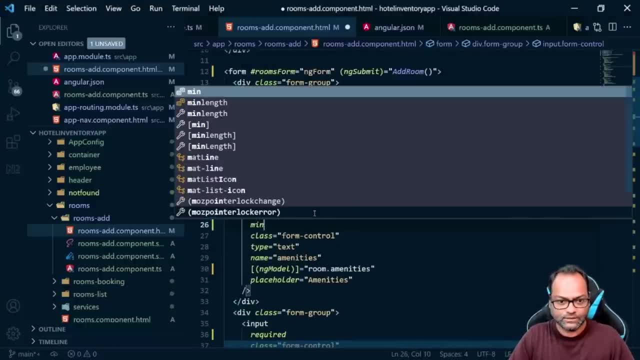 let's, let's go ahead and do that. let's, let's go ahead and do that. so here i'll we already have required, so here i'll we already have required, so here i'll we already have required, so i'll say min, so i'll say min. 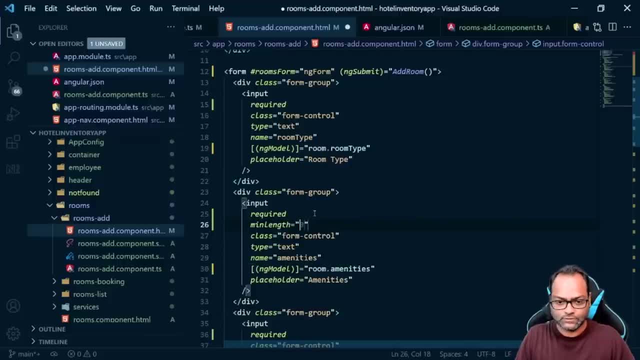 so i'll say: min length is equals to 50. uh, sorry, five is equals to 50. uh, sorry, five is equals to 50. uh, sorry, five. and we'll say max length and we'll say max length and we'll say max length is uh, is uh. 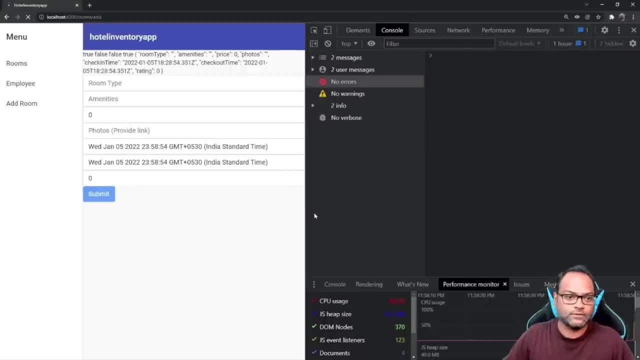 is: uh, let's make it 20 as of now. let's enter room, let's enter amenities. let's enter room, let's enter amenities. let's enter room, let's enter amenities, but let's not enter five characters. and but let's not enter five characters. and. 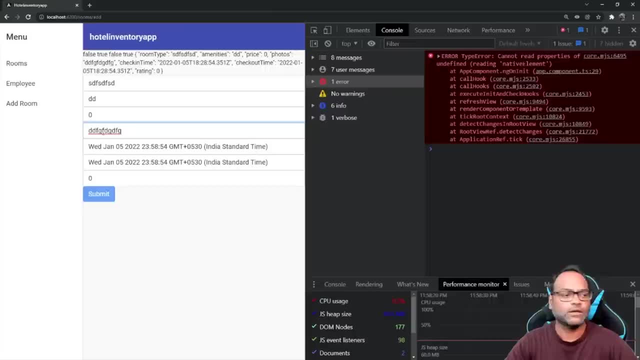 but let's not enter five characters. and let's enter, let's enter, let's enter amenities. you can see, uh, the form is still invalid. you can see, uh, the form is still invalid. you can see, uh, the form is still invalid. right, so, but the problem is here. 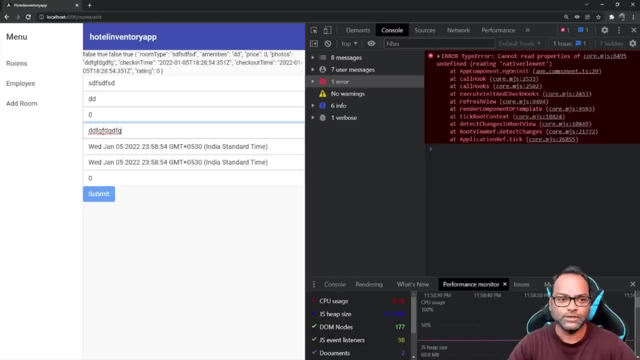 right so, but the problem is here. right so, but the problem is here. it actually introduces to uh us to it actually introduces to uh us to. it actually introduces to uh us to another issue. another issue, another issue. we are not able to display the errors. we are not able to display the errors. 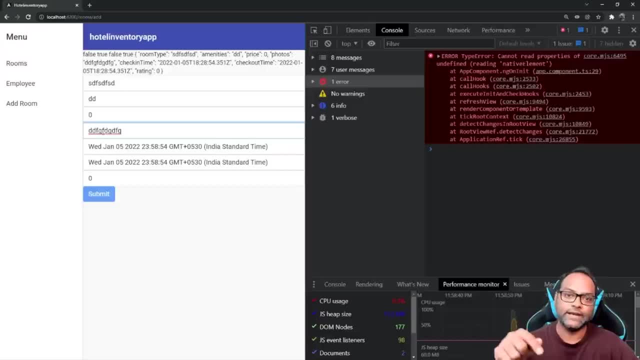 we are not able to display the errors based on what the actual error is based on what the actual error is, based on what the actual error is. we should, right now, we should display the. we should, right now, we should display the. we should, right now, we should display the masses saying: 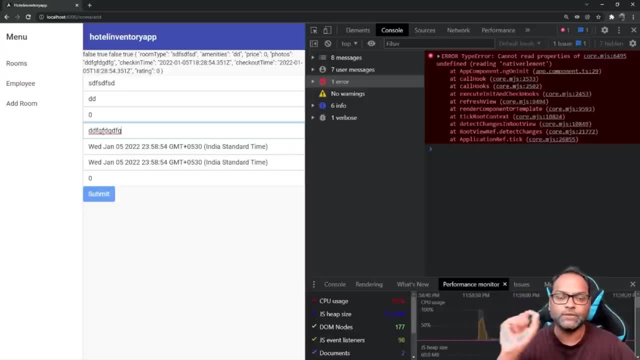 masses saying, masses saying okay, this particular, okay, this particular, okay, this particular form, form, form, value, or the amenities which you are value, or the amenities which you are value, or the amenities which you are trying to enter, is it should be minimum, trying to enter, is it should be minimum? 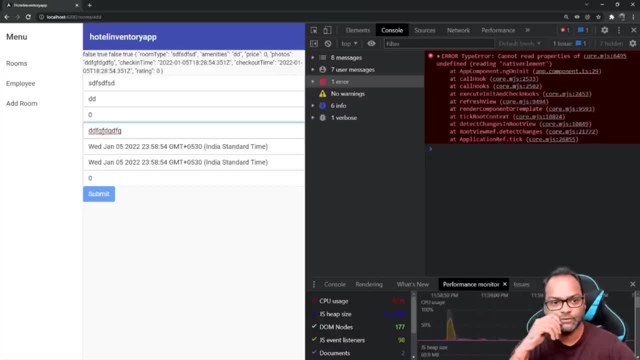 trying to enter is it should be minimum five characters, but it is not five characters, but it is not five characters, but it is not. the users will, of course, will be confused. the users will, of course, will be confused. the users will, of course, will be confused. what's going on here? 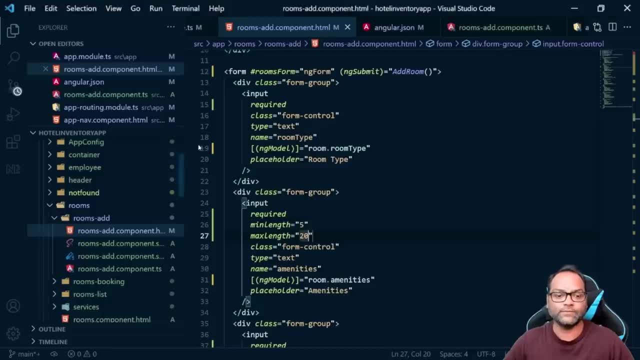 what's going on here? what's going on here? we should display the messages. so let's we should display the messages. so let's, we should display the messages. so let's go ahead and see how we can do that. go ahead and see how we can do that. 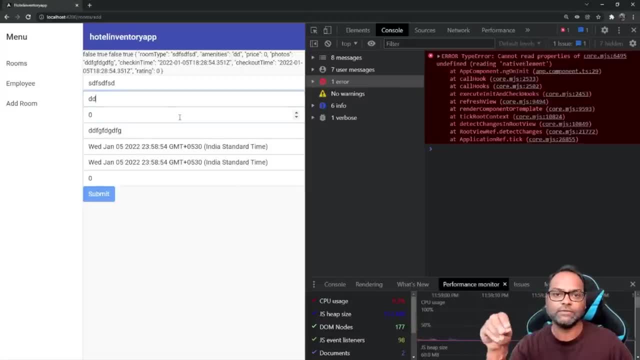 go ahead and see how we can do that. so this message is actually right now, or so this message is actually right now, or so this message is actually right now, or this error is actually available, right, this error is actually available, right, this error is actually available right now with the control. so here what we. 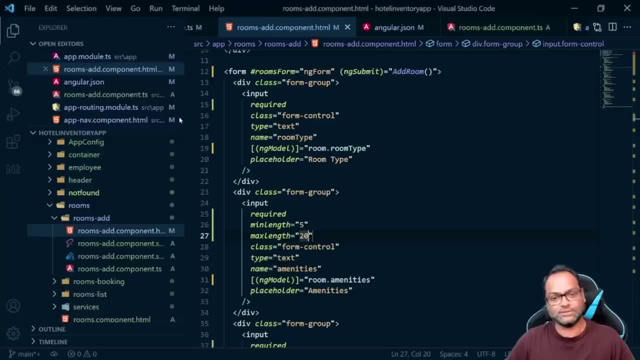 now with the control. so here, what we now with the control. so here, what we need is the access to control. how we can need, is the access to control. how we can need is the access to control how we can do that. yes, let's go ahead and see. 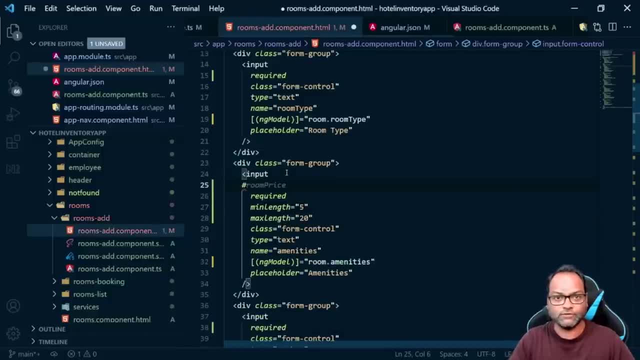 do that, yes, let's go ahead and see. do that, yes, let's go ahead and see, so to get the access to this control. we so to get the access to this control. we so to get the access to this control. we can say hash and whatever. uh, property. 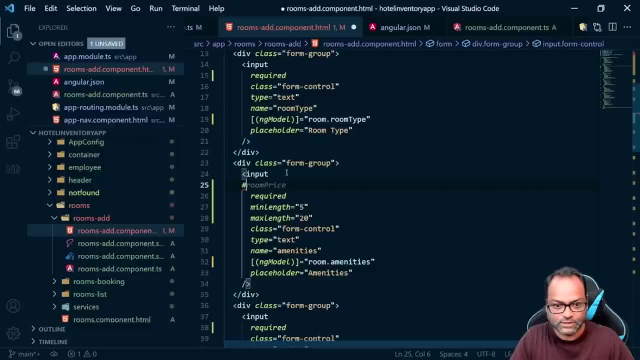 can say hash and whatever uh property can say hash and whatever uh property name you want to set it, so let's say uh name. you want to set it, so let's say uh name. you want to set it, so let's say, uh, this is amenities, right? so i'll say this: 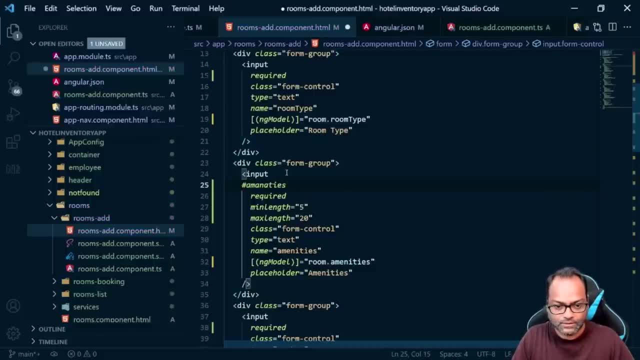 this is amenities, right, so i'll say this: this is amenities, right, so i'll say this: uh, amenities, it's a room amenities because it will. it's a room amenities because it will. it's a room amenities because it will conflict with another variable. conflict with another variable. 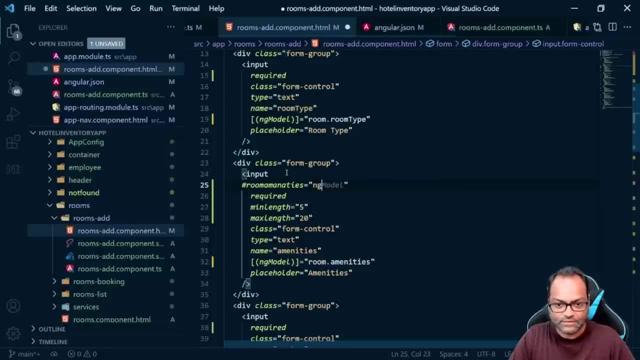 conflict with another variable room amenities is equals to you have to room amenities is equals to you have to room amenities is equals to you have to say ng model. remember this, say ng model, remember this, say ng model, remember this. and now let's go ahead and see. 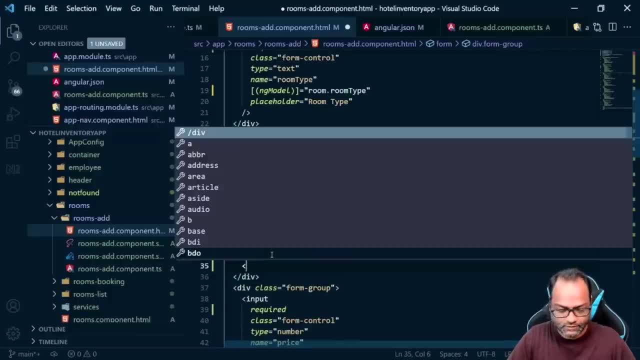 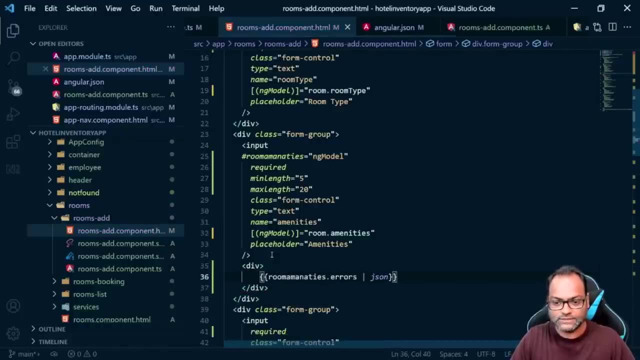 and now let's go ahead and see. and now let's go ahead and see, i'll place another, i'll place another, i'll place another, div, div, div. here, here, here, and we'll say, and we'll say, and we'll say: amenities, amenities, amenities, dot errors as json, let's go ahead and see. 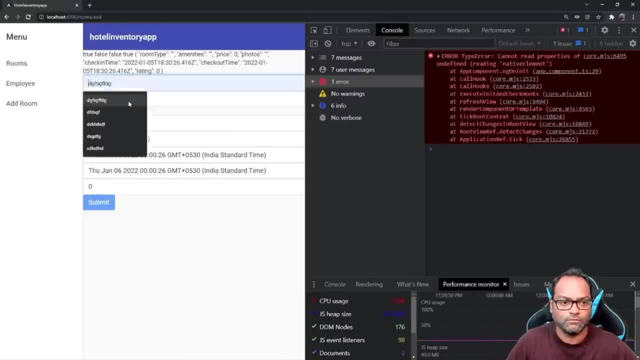 dot errors, as json, let's go ahead and see dot errors, as json, let's go ahead and see. so it says right now: uh, the error is so. it says right now: uh, the error is so. it says right now: uh, the error is required to, required to. 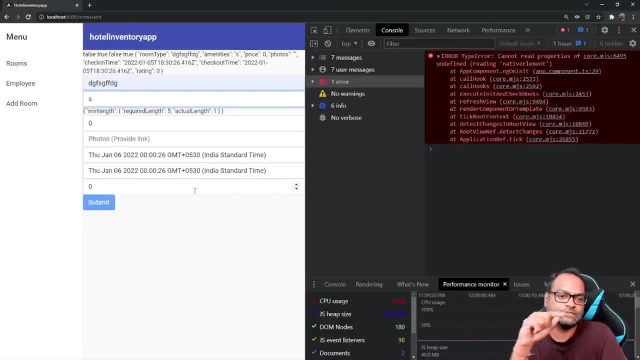 required to. but let's enter something right, so now. but let's enter something right, so now. but let's enter something right, so now. you can see it says min length required. you can see it says min length required. you can see it says min length required. length is five actually in this one, if i 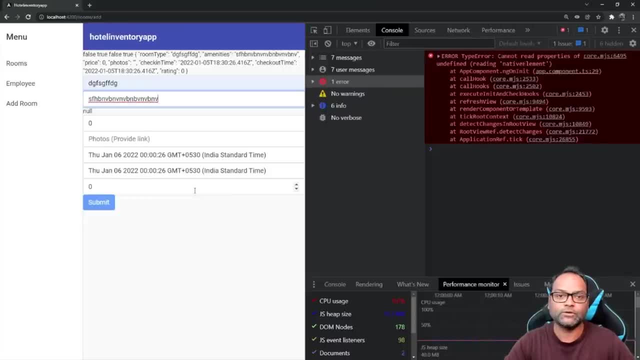 length is five actually in this one. if i length is five actually in this one, if i try to enter, try to enter, try to enter more than 20 character, i won't be able more than 20 character. i won't be able more than 20 character. i won't be able to do it because it is supported by the. 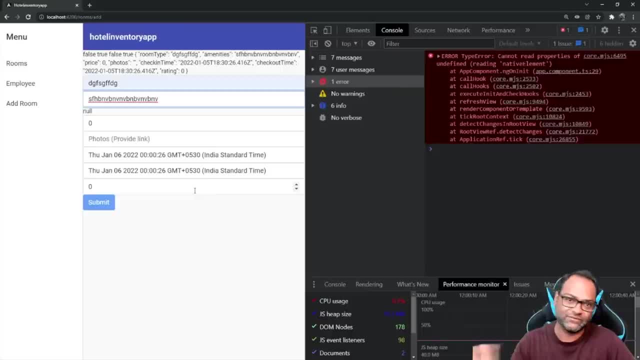 to do it because it is supported by the to do it because it is supported by the browsers: browsers, browsers. so, uh, it says okay, maximum length has. so, uh, it says okay, maximum length has. so, uh, it says okay, maximum length has reached, reached, reached 50 characters, or 20 characters, and we 50 characters or 20 characters and we 50 characters or 20 characters and we cannot enter more than 20.. so it it has cannot enter more than 20.. so it it has cannot enter more than 20.. so it it has stopped. i mean. 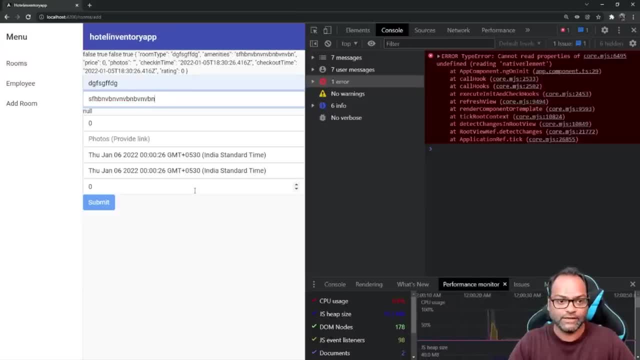 stopped. i mean stopped. i mean i'm right now, i'm still typing, but i'm, i'm right now, i'm still typing, but i'm, i'm right now, i'm still typing, but i'm not able to actually enter the values, not able to actually enter the values. 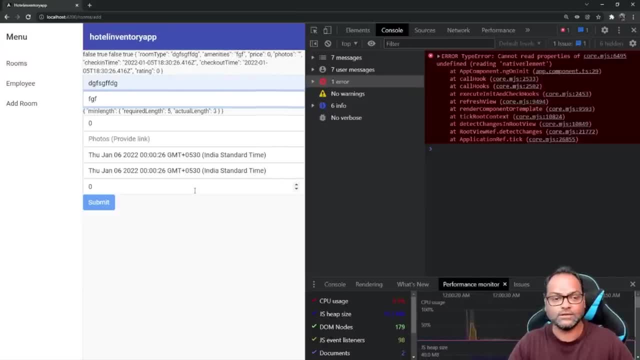 not able to actually enter the values. and if i go below five, it will again. and if i go below five, it will again. and if i go below five, it will again give me the same error. let's see how we give me the same error. let's see how we can display this as a message, right? so? 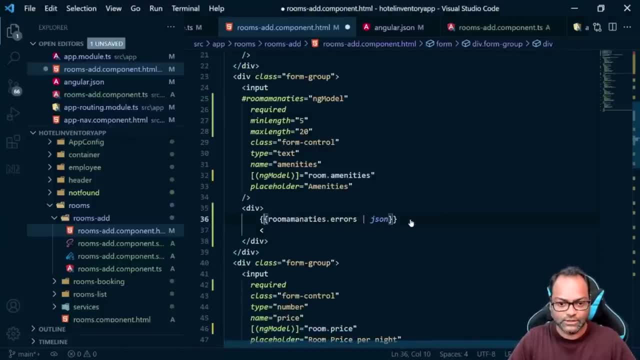 can display this as a message, right. so can display this as a message, right. so here here, here we can uh use. so here i'll just say we can uh use. so here i'll just say we can uh use. so here i'll just say uh first. 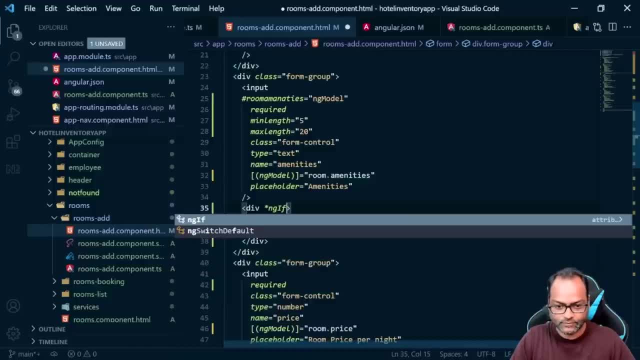 uh first. uh first star ng. if. if it has errors right now, you can also uh: if it has errors right now, you can also uh. if it has errors right now, you can also uh: do errors, dot which type of error we. do errors dot which type of error we. 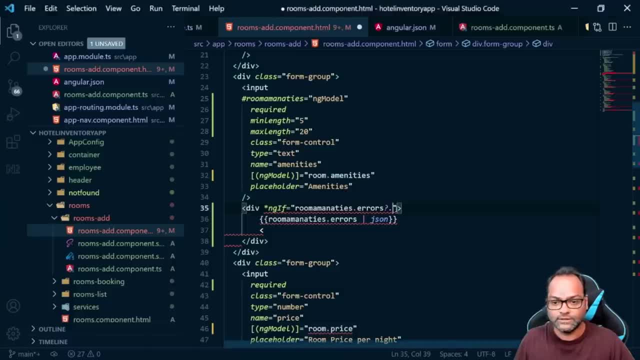 do errors, dot which type of error we are talking about. so here, let's say: if we are talking about so here, let's say: if we are talking about so here, let's say: if we talk about mean length, right, so i'll talk about mean length, right, so i'll. 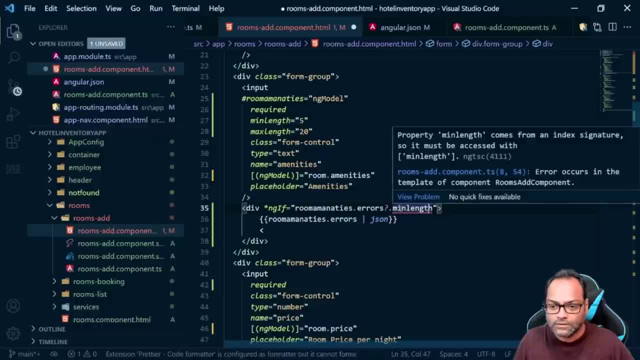 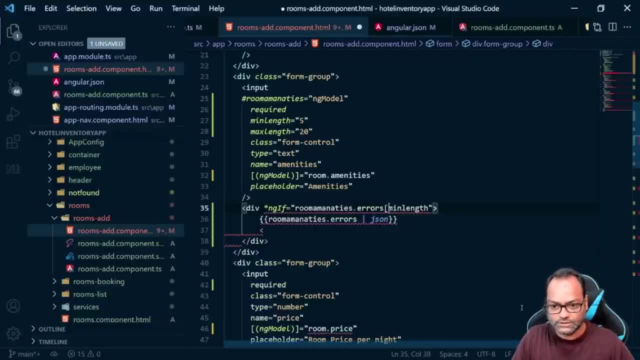 talk about mean length, right. so i'll say okay if uh the errors. okay, so it says it should be okay. so it says it should be okay, so it says it should be accessless this mill length and and and strange it is possibly. yeah, yeah, yeah. so i'm trying to access uh the, let's say 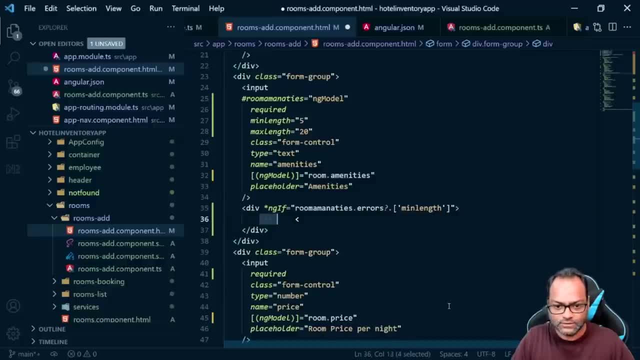 so i'm trying to access uh, the let's say so. i'm trying to access uh, the let's say it's. i'm saying, if it is it's, i'm saying, if it is it's, i'm saying if it is million error, million error, million error. so. 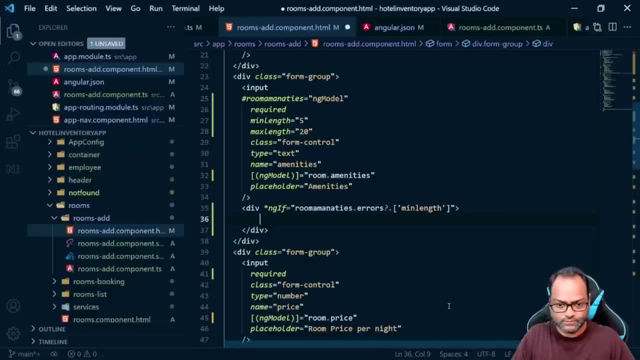 so what we can do is we can say what we can do, is we can say what we can do is we can say: uh, uh, uh, and we'll just add a class right so, and we'll just add a class right so, and we'll just add a class right so. class alert. 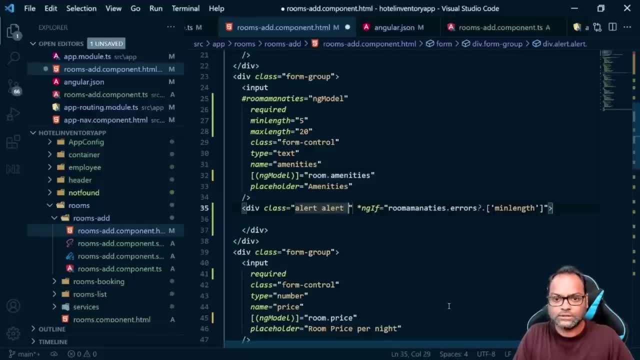 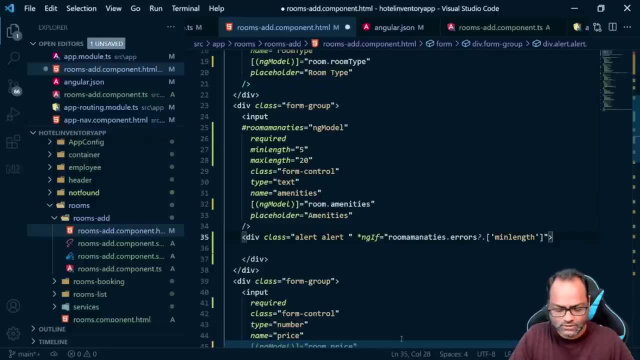 class alert, class alert alert. alert alert link. let's: what was this uh success? right so it. what was this uh success? right so it. what was this uh success? right so it should be alert, should be alert, should be alert, if i'm not wrong, danger. and let's say: 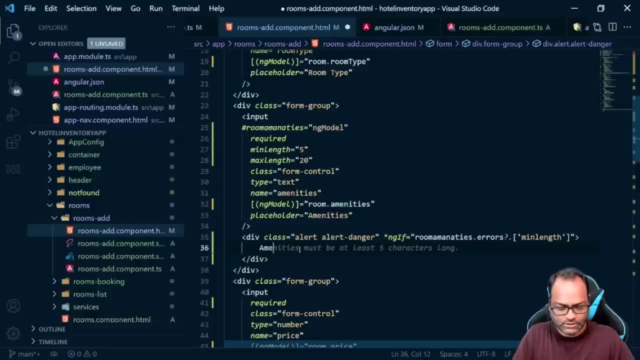 if i'm not wrong, danger, and let's say: if i'm not wrong, danger, and let's say: uh, emanate, please, emanate, please, emanate, please, should, should, should be five cars. be five cars, be five cars. minimum, minimum, minimum or should be minimum, or should be minimum. 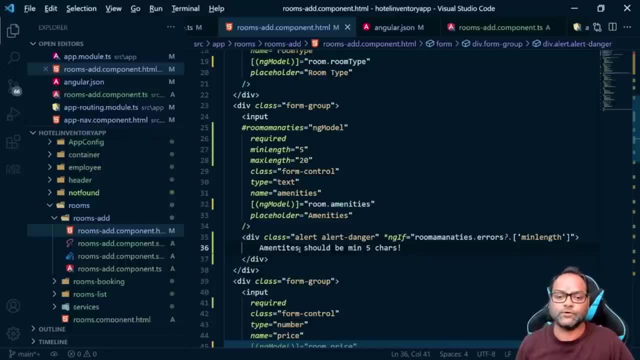 or should be minimum, minimum five casts. so this is the minimum five casts. so this is the minimum five casts. so this is the information we want to show. information, we want to show information we want to show. let's go ahead and see. let's go ahead and see. 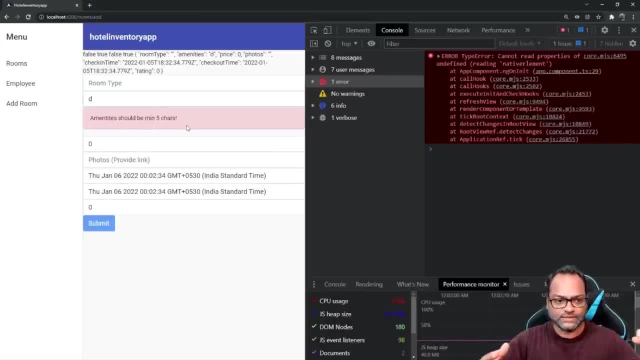 let's go ahead and see: let's enter one character and you have let's enter one character and you have let's enter one character and you have the message available here. it says: i the message available here. it says i the message available here. it says i mean it should be five characters. 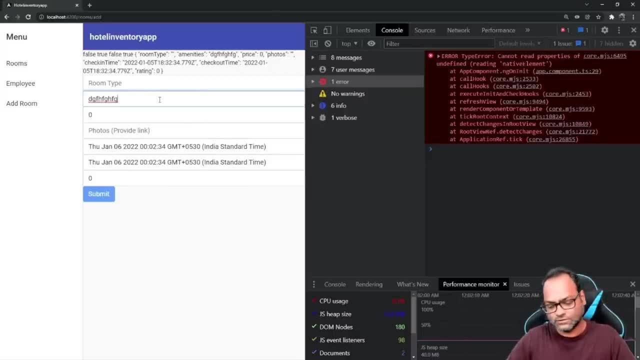 mean it should be five characters, mean it should be five characters and as soon as we, and as soon as we, and as soon as we go beyond five characters, the error is go beyond five characters. the error is go beyond five characters. the error is gone. but yeah, so this is. 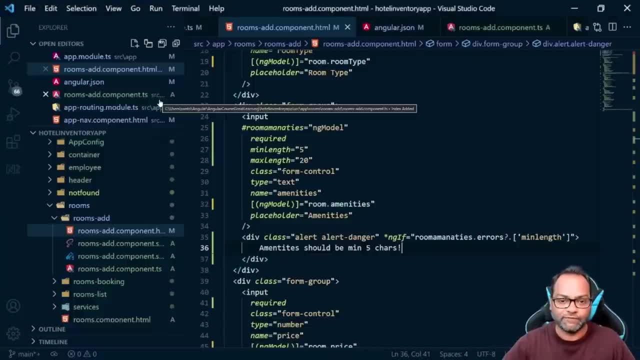 how you can display the errors, on how you can display the errors, on how you can display the errors on control level, control level, control level- so we have this, and of course you can. so we have this, and of course you can. so we have this, and of course you can also say errors. 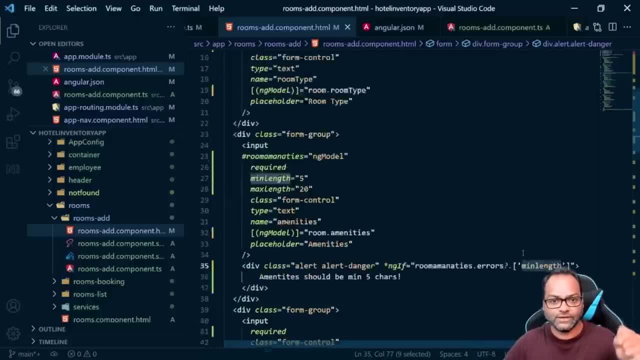 also say errors, also say errors of required, and then you can also say of required, and then you can also say of required, and then you can also say, okay, this amenities is required, okay, this amenities is required, okay, this amenities is required, this room type is required, all on your. 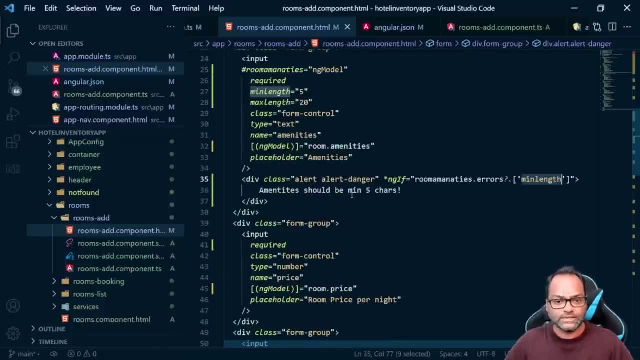 this room type is required. all on your. this room type is required. all on your control level. that is also possible control level. that is also possible control level. that is also possible. so we saw min length and max length. so we saw min length and max length. so we saw min length and max length. what's next? what's next? so we have uh. 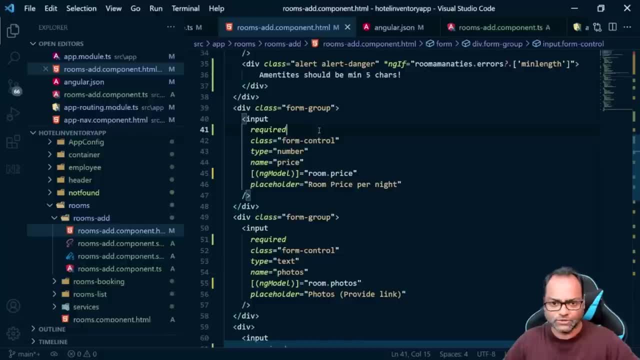 what's next? what's next? so we have, uh, what's next? what's next? so we have, uh, the min and max, the min and max, the min and max as well. i'm not sure if it still works as well. i'm not sure if it still works. 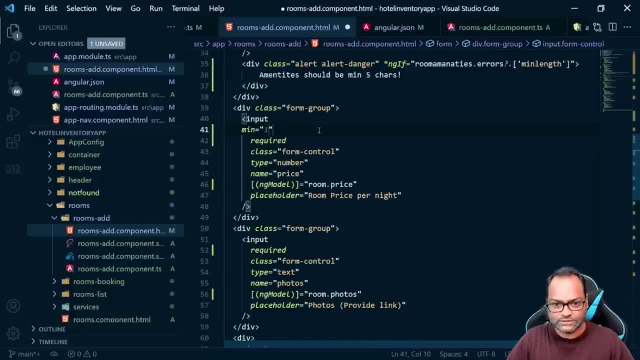 as well. i'm not sure if it still works, but let's see, but, let's see, but let's see. so it's a mean uh which is so. it's a mean uh which is so. it's a mean uh which is one, one, one and max, which is. 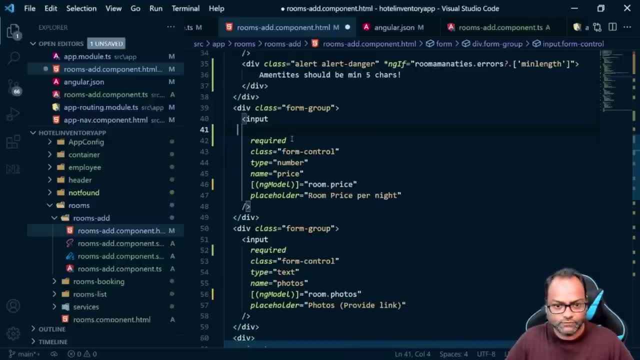 and max which is and max which is five. let's see five. let's see five. let's see: this is okay. i'll not do it here. let's: this is okay. i'll not do it here. let's: this is okay. i'll not do it here, let's do it for. 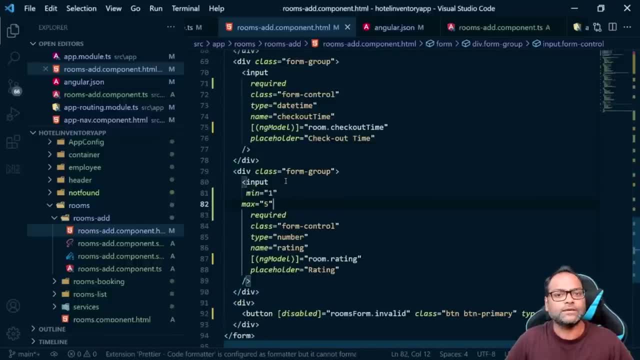 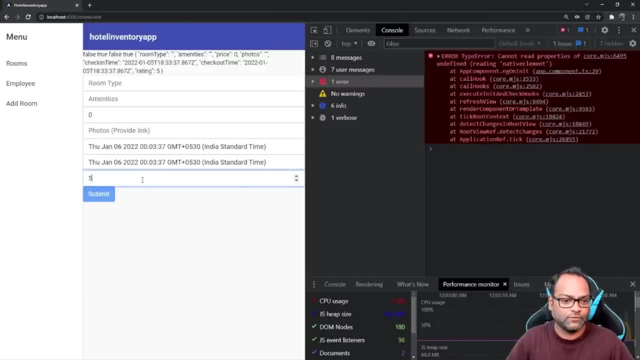 do it for. do it for one, two, three, four, five. now i won't be one, two, three, four, five. now i won't be one, two, three, four, five. now i won't be able to actually go beyond five, able to actually go beyond five, able to actually go beyond five. i'm just still, still pressing, uh, the up. 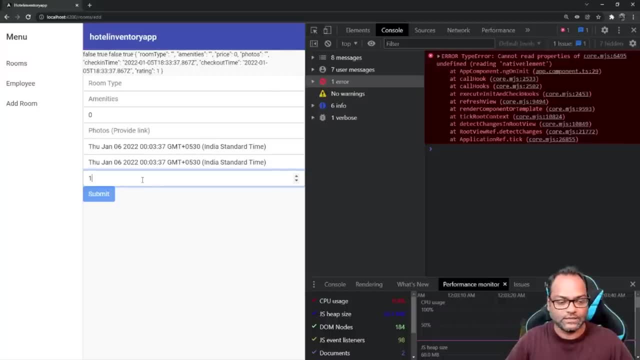 i'm just still still pressing uh the up. i'm just still still pressing uh the up, key, but i'm not able to go key, but i'm not able to go key, but i'm not able to go. so let's go ahead and say uh else is zero, and let's enter all the. 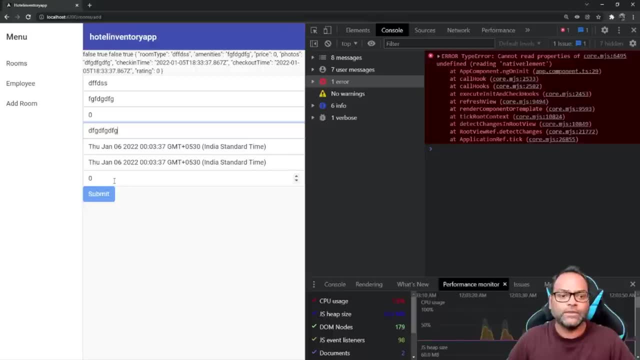 else is zero and let's enter all the else is zero and let's enter all the other details, other details, other details and photos, but we are still not able to and photos, but we are still not able to and photos, but we are still not able to submit as soon as we move to one, because 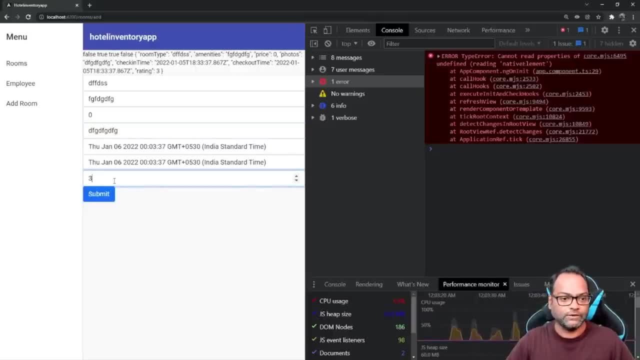 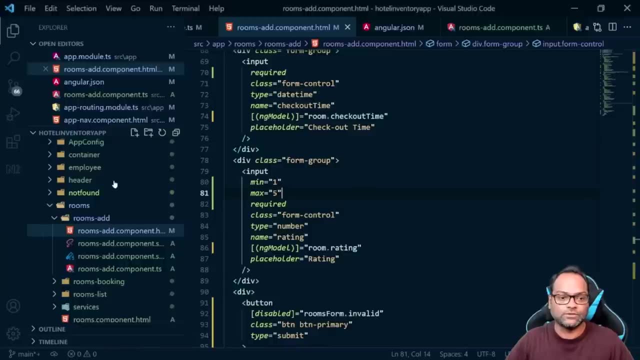 submit as soon as we move to one, because submit as soon as we move to one, because so this is how you can do with min, and so this is how you can do with min, and so this is how you can do with min and max. so we learned about required. 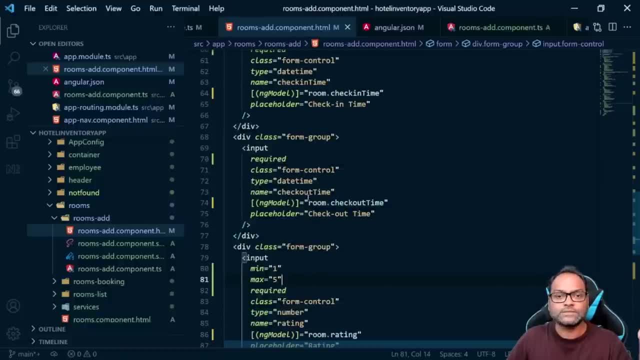 max. so we learned about required max. so we learned about required million max length. uh, then we talk million max length. uh, then we talk million max length. uh, then we talk about min and max. what else what other about min and max? what else what other about min and max? what else, what other validators which we have in html5? 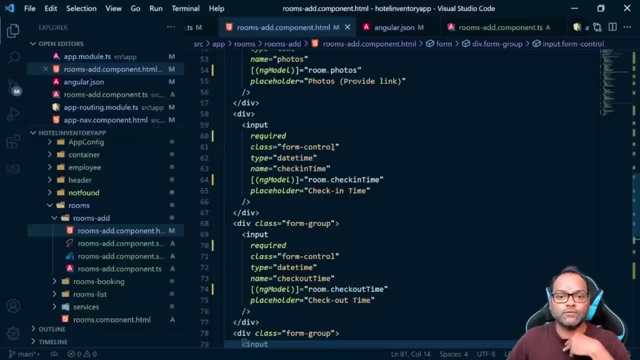 validators which we have in html5, validators which we have in html5, so we also have a validator for. so we also have a validator for. so we also have a validator for email, email, email. so email, of course you can mark any. so email, of course you can mark any. 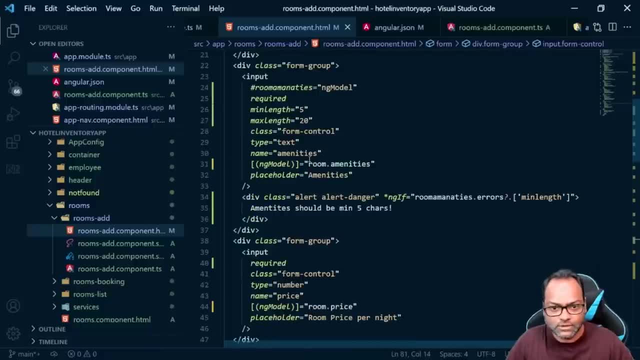 so email. of course, you can mark any property as email and it will be property as email, and it will be property as email and it will be considered as an email. so let's try. considered as an email, so let's try. considered as an email. so let's try. right now, we don't have anything for. 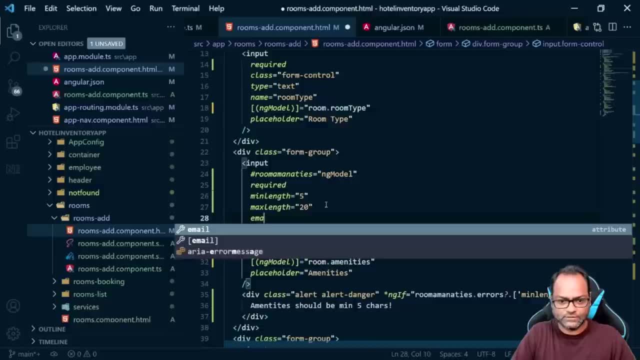 right now we don't have anything for right now we don't have anything for email but email, but email. but just just just for an example, right so we just make it for an example. right so we just make it for an example, right so we just make it email. 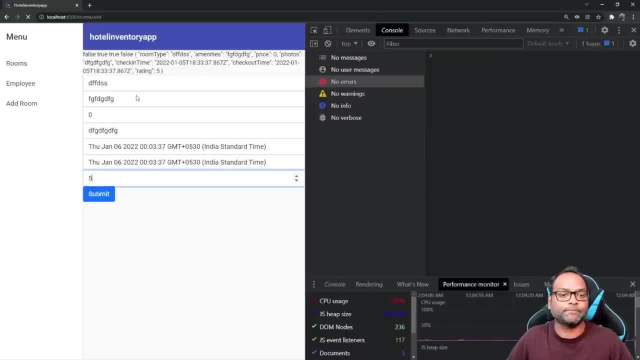 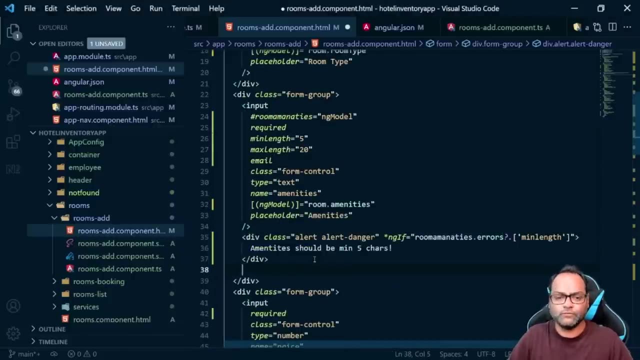 email, email. um, i think email is enough. let's see and let's display all the errors. and let's display all the errors. and let's display all the errors. otherwise we won't be able to figure out, otherwise we won't be able to figure out, otherwise we won't be able to figure out right. 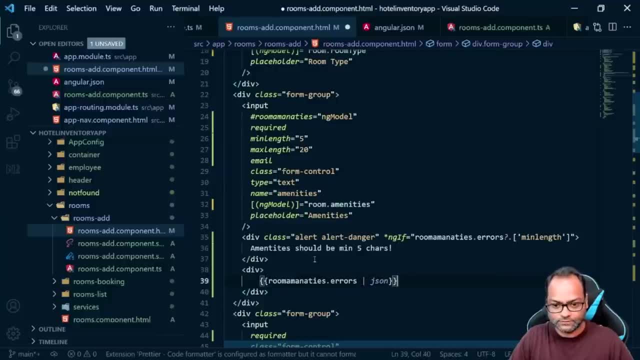 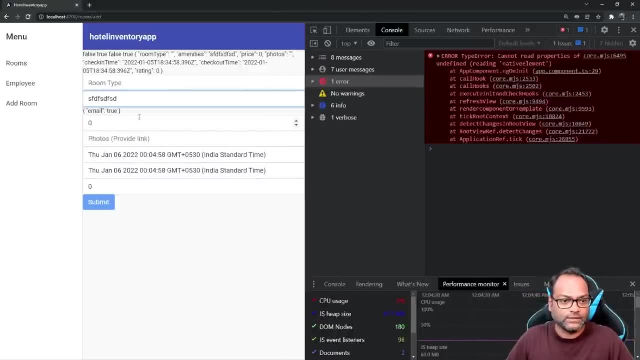 right, right, which kind of error is this? so you can see, uh, it says okay, min length. so you can see, uh, it says okay, min length. so you can see, uh, it says okay, min length, max length, max length, max length. and then now it says it's, uh, there is. 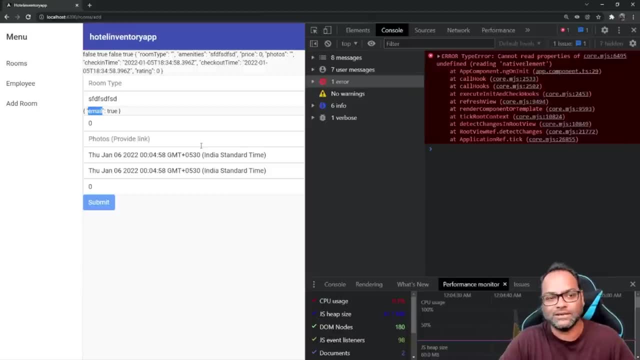 and then now it says it's: uh, there is. and then now it says it's: uh, there is this particular text. whatever you have this particular text, whatever you have this particular text, whatever you have entered, it's not an email entered, it's not an email entered, it's not an email. so if i go ahead and say: add the rate, 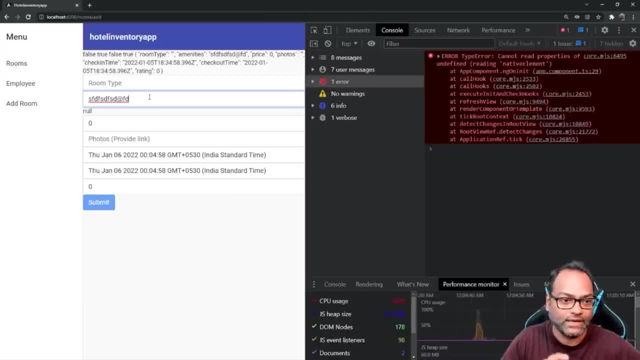 so if i go ahead and say add the rate, so if i go ahead and say add the rate, now we have actually uh a valid email. now we have actually uh a valid email. now we have actually uh a valid email. that's as per the html5. 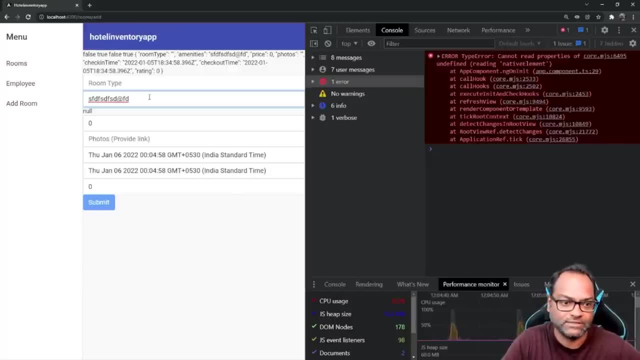 that's as per the html5. that's as per the html5 validation validator. this is an actual validation validator. this is an actual validation validator. this is an actual valid html. sorry, valid email. valid html. sorry, valid email. valid html. sorry, valid email. so this is email and. 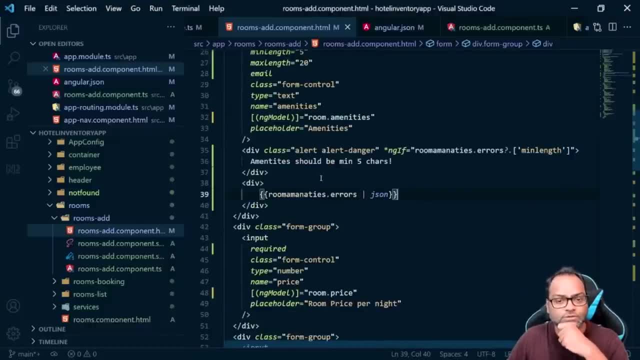 so this is email, and so this is email and what other? so, uh, there is also something, what other? so, uh, there is also something, what other? so, uh, there is also something known as format, so format takes regex known as format. so format takes regex known as format. so format takes regex. so you can actually 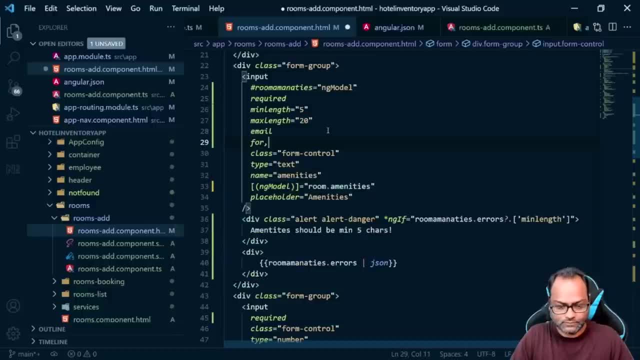 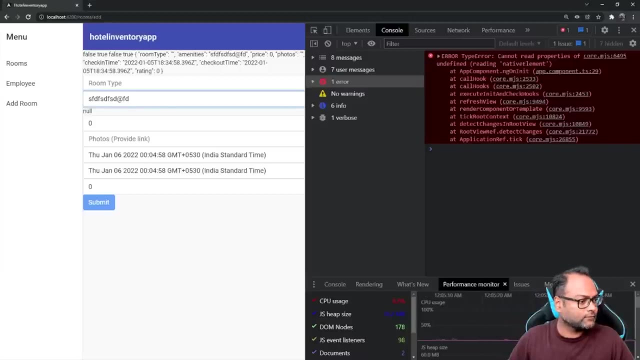 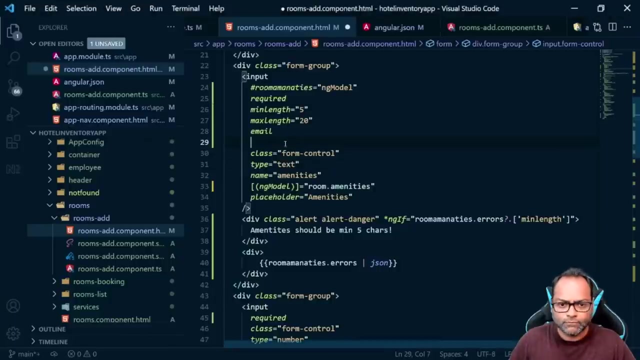 so you can actually, so you can actually use, use. ah okay, sorry, it's not uh. so the next. ah okay, sorry, it's not uh. so the next. ah okay, sorry, it's not uh. so the next validator which we are validator, which we are validator, which we are we're going to talk about, it's known as 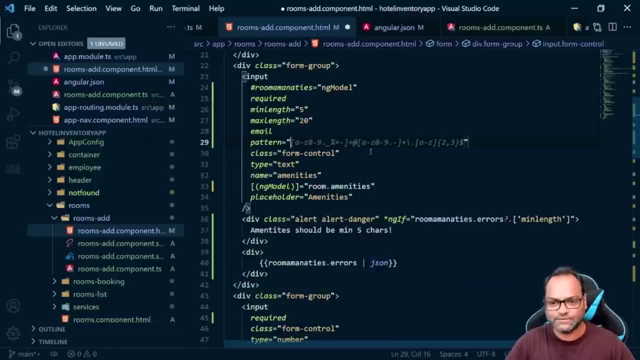 we're going to talk about. it's known, as we're going to talk about, it's known as pattern, so pattern is something where pattern, so pattern is something where pattern, so pattern is something where you can provide a regular expression for. you can provide a regular expression for. 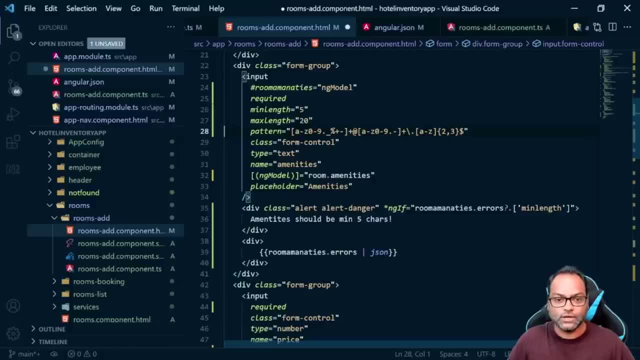 you can provide a regular expression, for example: i don't know what this regex is. example: i don't know what this regex is. example: i don't know what this regex is. thanks to our thanks to our thanks to our github copilot, which gave me this regex. 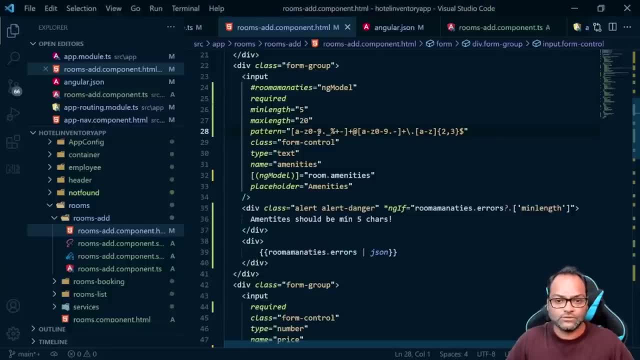 github copilot, which gave me this regex. github copilot, which gave me this regex for some some reason. so let's see what- for some some reason. so let's see what, for some some reason. so let's see what this pattern is. so here i can just 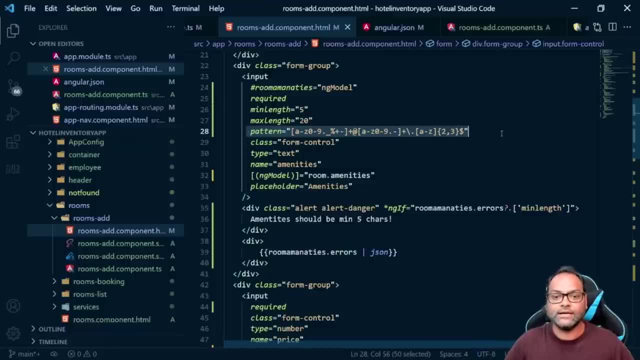 this pattern is so here i can just this pattern is so here i can just provide this pattern, a regular, provide this pattern, a regular. provide this pattern, a regular expression and my text. whatever i enter expression and my text, whatever i enter expression and my text, whatever i enter, will be actually. 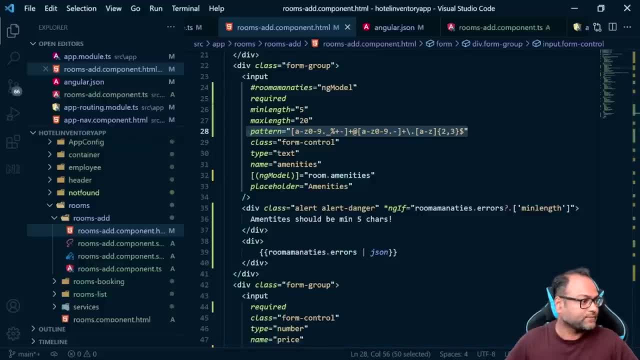 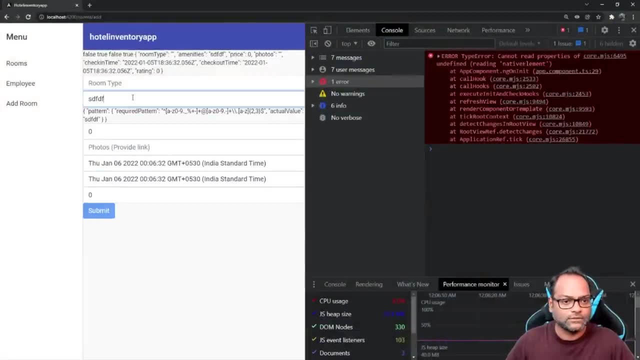 will be actually will be actually validated against this pattern. so this validated against this pattern. so this validated against this pattern. so this is regular expression. let's see so it says okay, required. let's see so it says okay, required. let's see so it says okay, required. pattern is this? i'm not sure what. 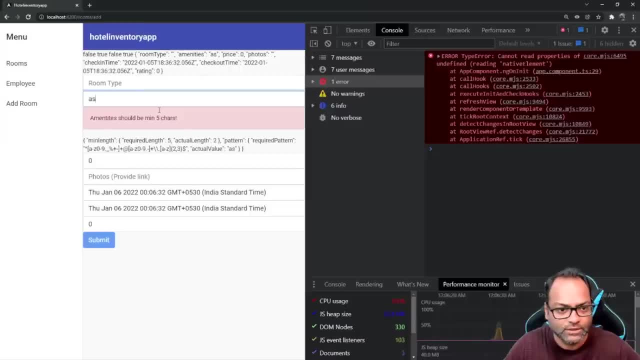 pattern is this? i'm not sure. what pattern is this? i'm not sure what required pattern is. it starts from a to required pattern. is it starts from a to required pattern? is it starts from a to z? and then there are number z and then there are number. 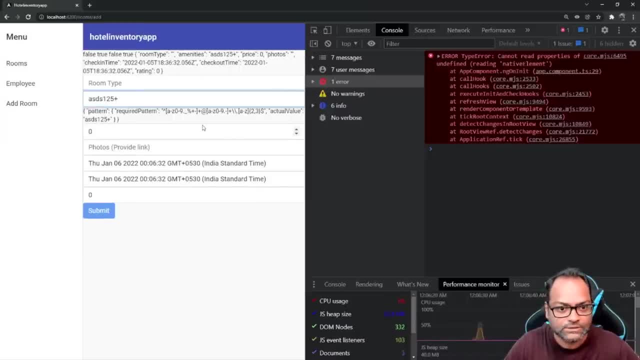 z, and then there are number, so one, two, three, uh, then there is plus. so one, two, three, uh, then there is plus, so one, two, three, uh, then there is plus at the rate, at the rate, at the rate. okay, and i still don't understand what. okay, and i still don't understand what. 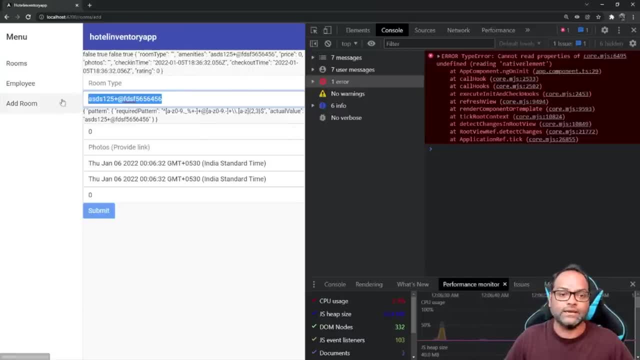 okay and i still don't understand what this pattern is. probably we can search this pattern is probably we can search this pattern is probably we can search for this regular expression and see for this regular expression and see for this regular expression and see, but yeah, you can provide any regular. 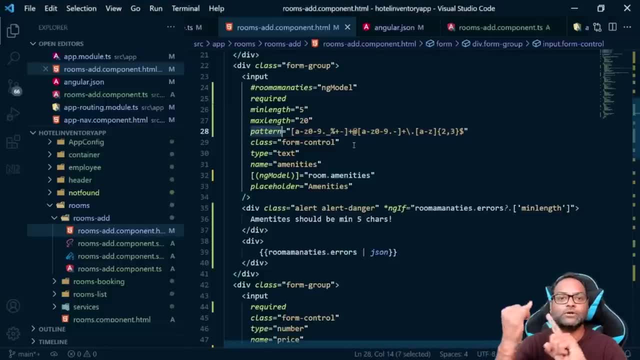 but yeah, you can provide any regular. but yeah, you can provide any regular expression as a pattern, and this will be expression as a pattern, and this will be expression as a pattern, and this will be validated. so we validated, so we validated, so we learn about required million max length. 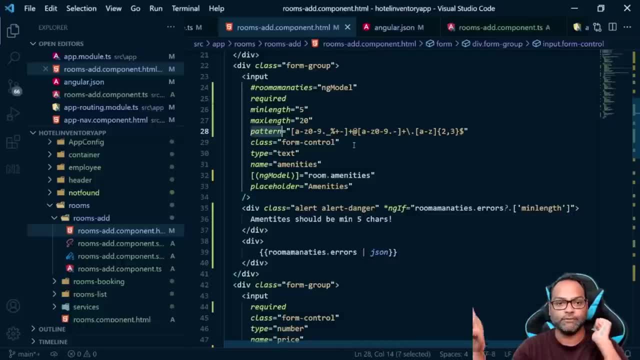 learn about required million max length. learn about required million max length. min map min max. uh, we talked about email. min map min max. uh, we talked about email. min map min max. uh, we talked about email. we talked about, we talked about, we talked about pattern. so these are different validators. 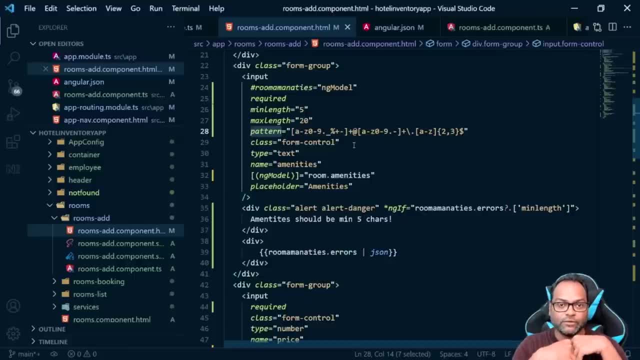 pattern. so these are different validators pattern. so these are different validators which we can use, which we can use, which we can use while working with template driven. while working with template driven. while working with template driven- sorry while working with template driven. sorry, while working with template driven. 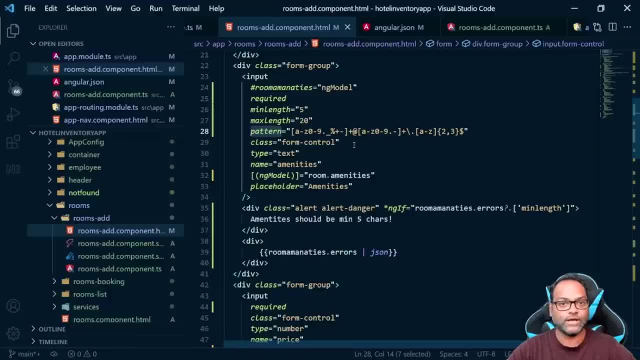 sorry, while working with template driven forms and all these are built-in forms. and all these are built-in forms and all these are built-in validators. you don't have to do anything. validators, you don't have to do anything. validators: you don't have to do anything extra to use them. 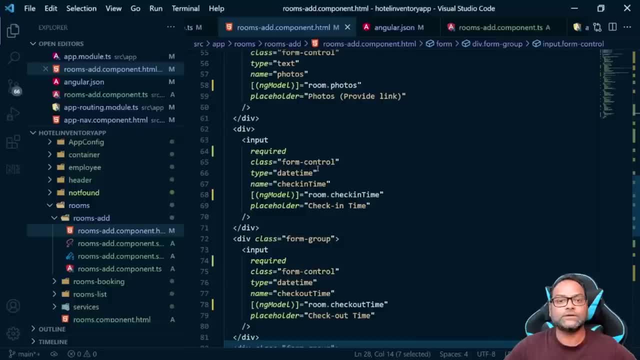 extra to use them extra. to use them. so this, so this, so this it. this is it from the required it. this is it from the required it. this is it from the required validated part. what we covered is we validated part. what we covered is we validated part. what we covered is: we also saw how we can. 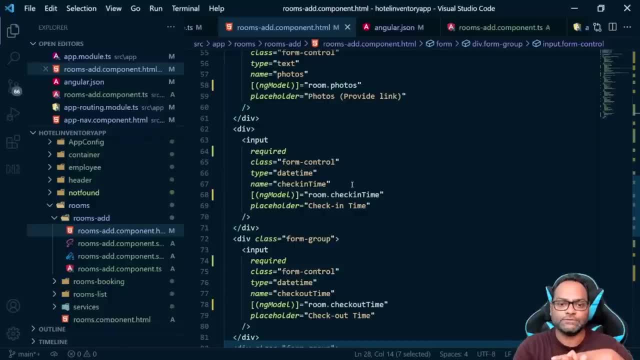 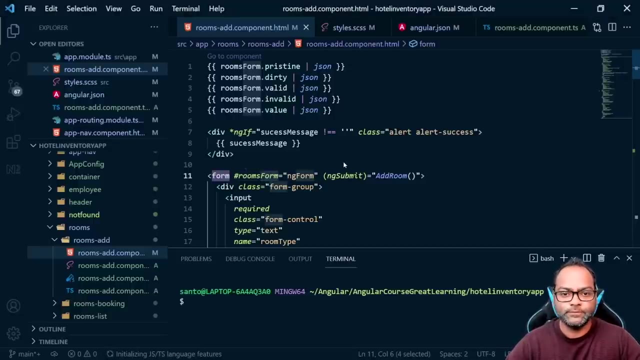 also saw how we can, also saw how we can in this video we are going to talk in this video. we are going to talk in this video. we are going to talk about few things, about few things, about few things. uh, we talked about valid, invalid, but we 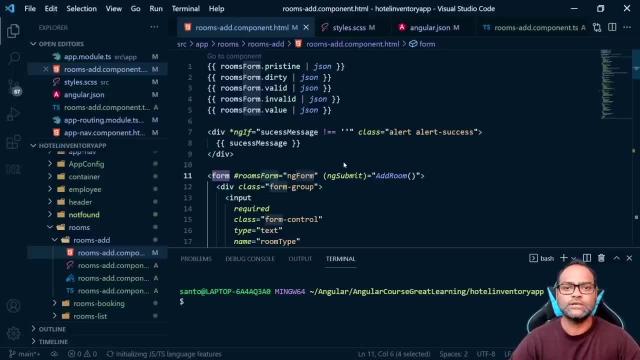 uh, we talked about valid invalid, but we, uh, we talked about valid invalid, but we didn't test, didn't test, didn't test- pristine and dirty. so let's talk about pristine and dirty. so let's talk about pristine and dirty. so let's talk about these two states, because they are really 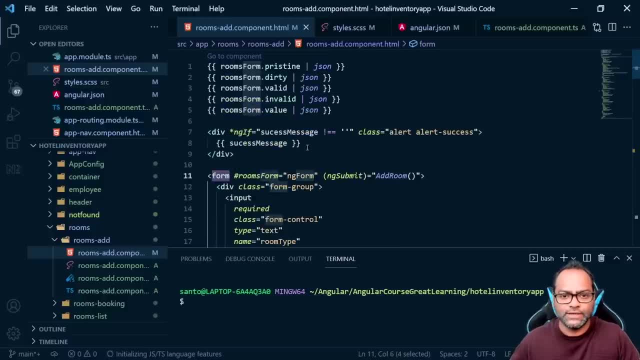 these two states, because they are really these two states, because they are really important to understand, important to understand, important to understand, and uh, to show you an example, let me and uh to show you an example. let me and uh to show you an example. let me just open the. 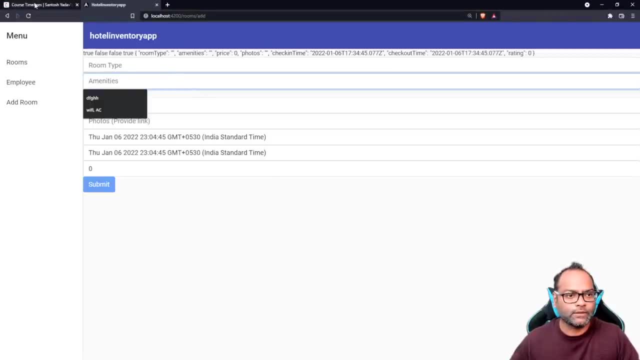 just open the, just open the. um, yeah, let me just open the. yeah, let me just open the. yeah, let me just open the uh view and you can see here right now: uh view. and you can see here right now: uh view. and you can see here right now. this required true error is already there. 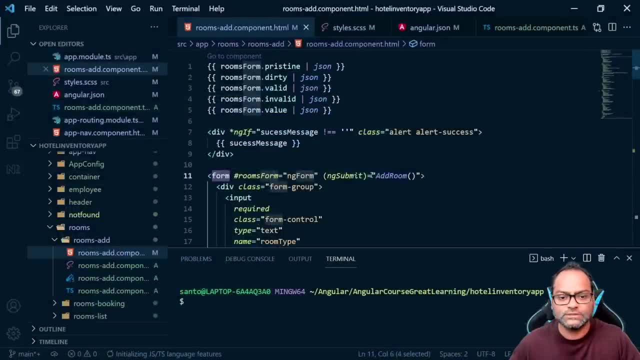 this required true error is already there. this required true error is already there, right? so one second let's go back to our right. so one second let's go back to our right. so one second let's go back to our code base. code base, code base and. 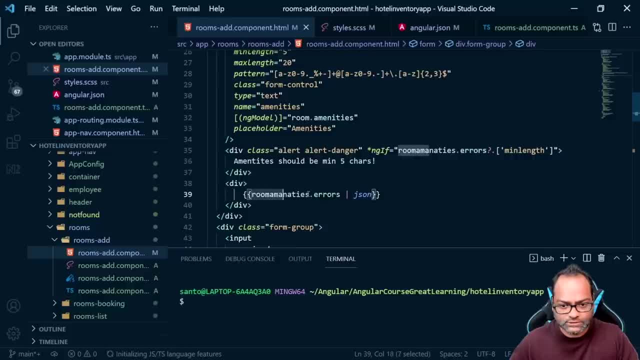 and and this errors. so if i do something like this, errors. so if i do something like this, errors. so if i do something like this, this, this div, div, div, star ng, if star ng, if star ng, if errors, dot, dot, dot, required, required, required, required, dot, required. and here let's say: 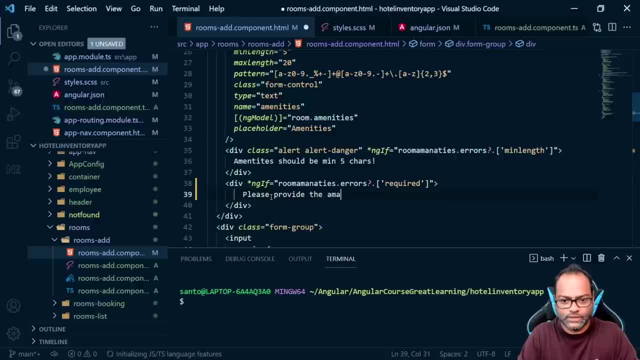 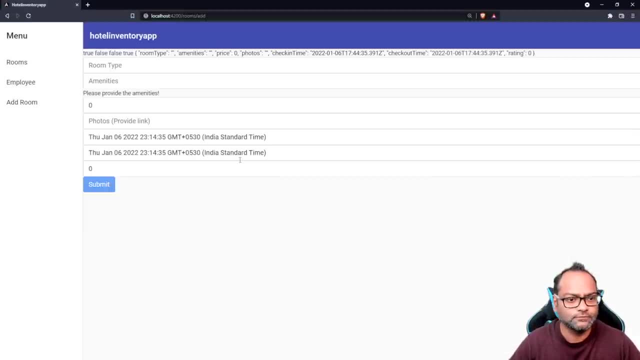 please, please, please, provide, provide, provide the amenities. let's see the output so you can see. this error message is so you can see. this error message is so you can see. this error message is available here, of course, and we have not available here, of course, and we have not. 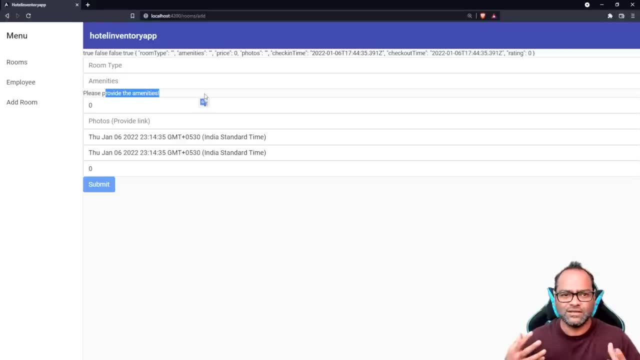 available here, of course, and we have not provided the class. but yeah, this error provided the class. but yeah, this error provided the class. but yeah, this error message is available here. but message is available here. but message is available here. but as a user, i haven't actually touched the. 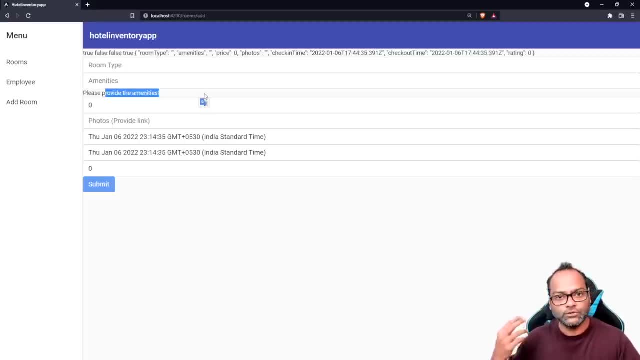 as a user, i haven't actually touched the. as a user, i haven't actually touched the control, or i haven't entered anything- control, or i haven't entered anything- control, or i haven't entered anything. so using pristine, you can actually avoid. so, using pristine, you can actually avoid. 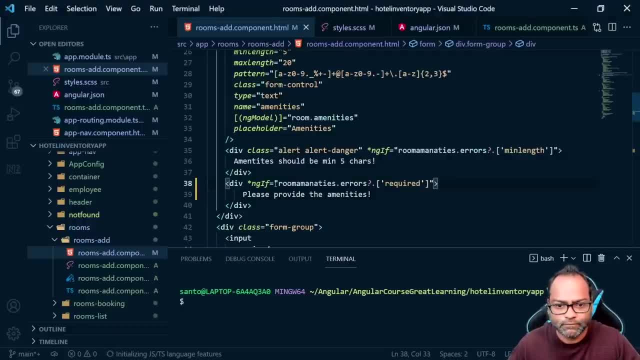 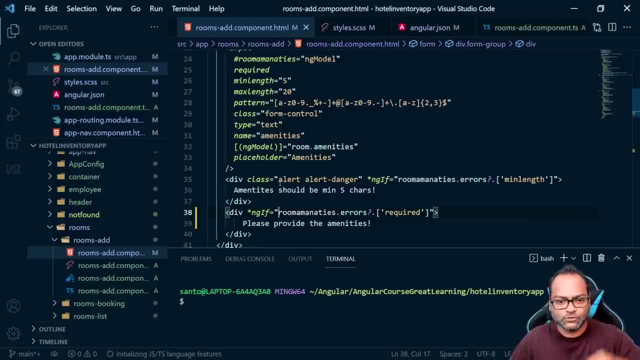 so, using pristine, you can actually avoid something like this. so you can do here, here, here, remember this, this property is available. remember this, this property is available. remember this: this property is available on form as well as control. so i i'm on form as well as control, so i i'm. 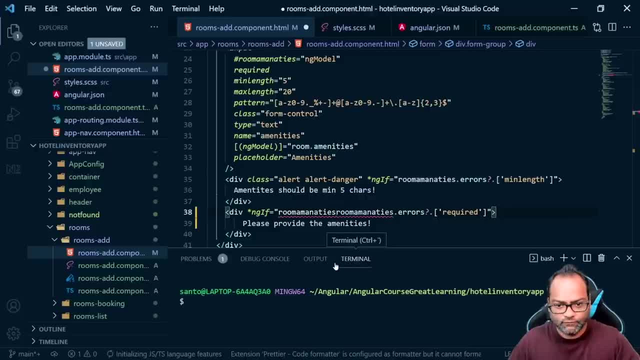 on form as well as control. so i i'm going to use it on the control, so i can going to use it on the control, so i can going to use it on the control so i can say, say, say, if, if, if, dot, dot, dot, pristine, pristine. 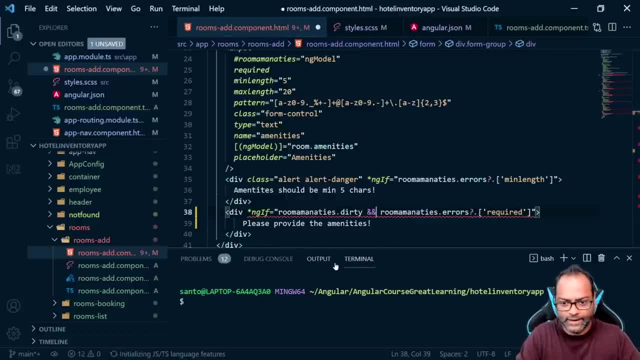 pristine, so let's say dirty, so let's say dirty, so let's say dirty. and this too. so i'm combining and this too, so i'm combining, and this too, so i'm combining these two properties, but let's say let's, these two properties, but let's say let's. 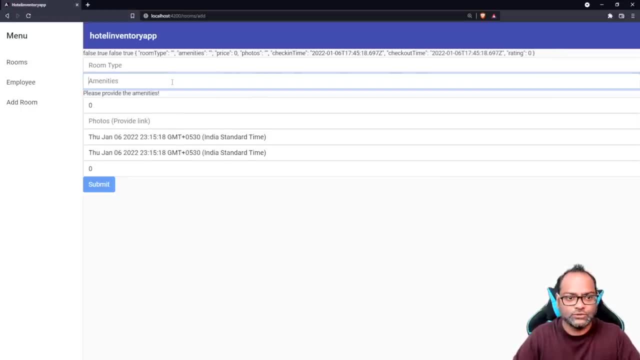 these two properties. but let's say, let's see what we are going to achieve using. see what we are going to achieve using. see what we are going to achieve using this right, this right, this right. so you can see i don't have the error. so you can see i don't have the error. 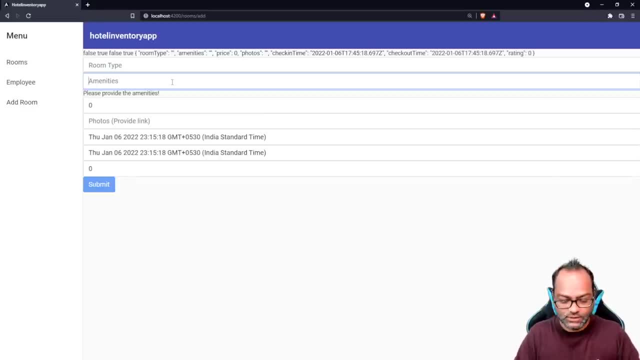 so you can see, i don't have the error when the view was available at the first, when the view was available at the first, when the view was available at the first time. so i'm providing time, so i'm providing time, so i'm providing the ability to. 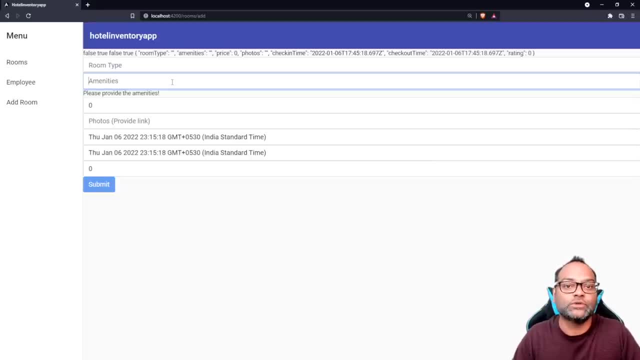 the ability to the ability to enter some text. enter some text, enter some text before i go ahead and show the error. so, before i go ahead and show the error, so before i go ahead and show the error, so in case i remove it, in case i remove it. 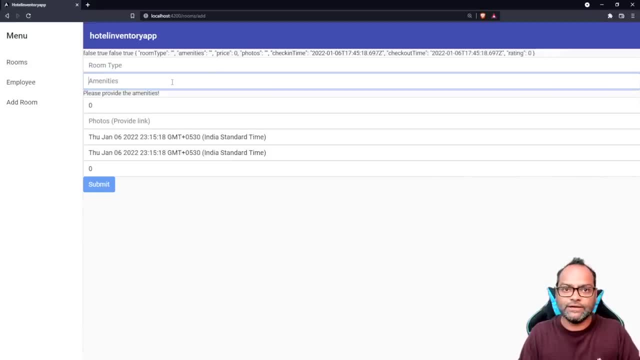 in case i remove it, i delete the entire thing. i will get this. i delete the entire thing. i will get this. i delete the entire thing. i will get this error, which is really valid right. i error which is really valid right. i error which is really valid, right. i mean. 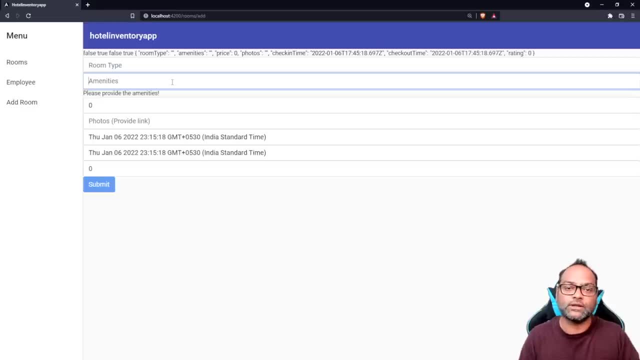 mean mean, as i have entered something, and then i, as i have entered something, and then i, as i have entered something, and then i removed it. i should show this particular, removed it. i should show this particular, removed it. i should show this particular error message. so how does pristine and 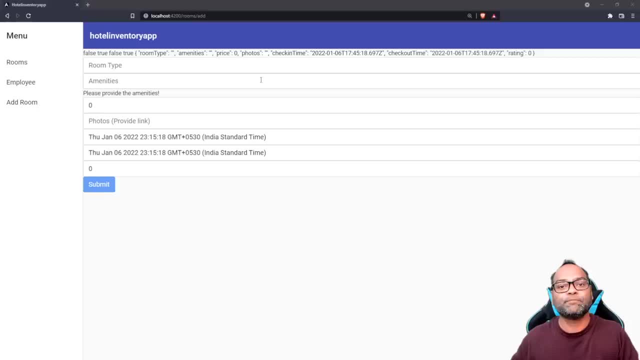 error message. so how does pristine? and error message. so how does pristine? and dirty helps? so let me talk about these. dirty helps. so let me talk about these dirty helps. so let me talk about these two properties, two properties, two properties. so pristine, so pristine. so pristine always means fresh state to your form. 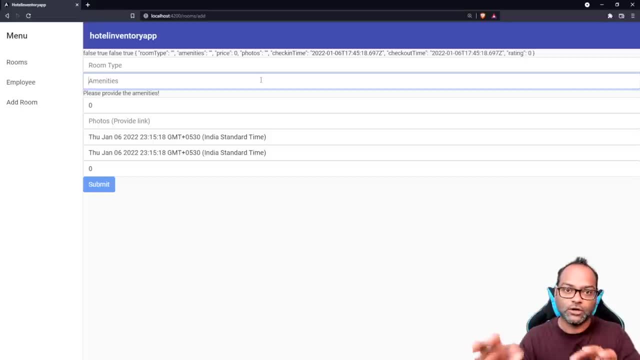 always means fresh state to your form. always means fresh state to your form. control- it means control. it means control. it means no one has actually touched your form. so no one has actually touched your form, so no one has actually touched your form. so let me just refresh this page. 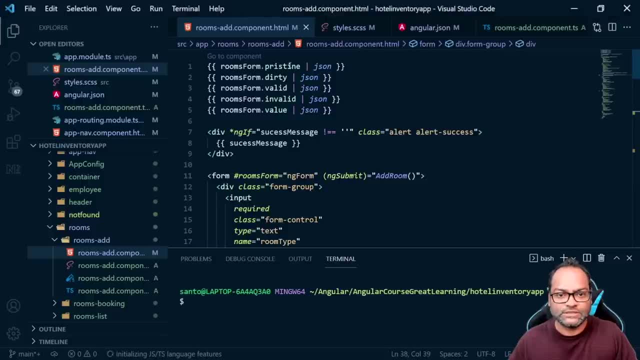 let me just refresh this page. let me just refresh this page and you can see the pristine value is and you can see the pristine value is and you can see the pristine value is true. why true? why true? why i'm saying this is a pristine? because of 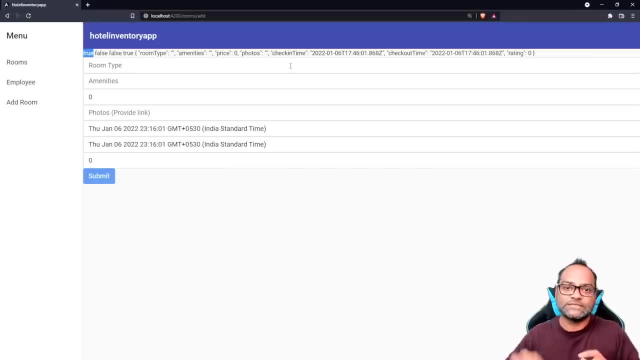 i'm saying this is a pristine because of. i'm saying this is a pristine because, of course, we have actually logged pristine course. we have actually logged pristine course. we have actually logged pristine first. so pristine is frustrated as soon first. so pristine is frustrated as soon first. so pristine is frustrated as soon as i interact with any control inside. 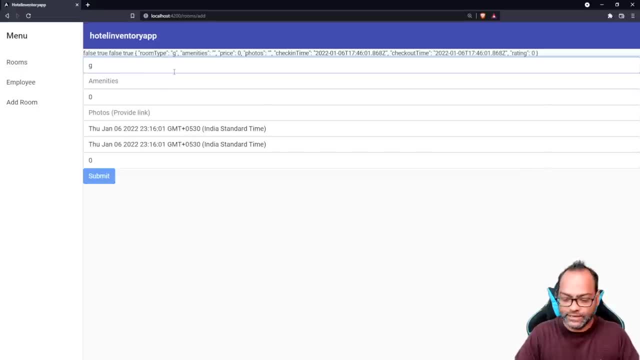 as i interact with any control inside, as i interact with any control inside this form, let's do that it becomes false. this form, let's do that it becomes false. this form, let's do that it becomes false and it will be false. remember valid and it will be false. remember valid. 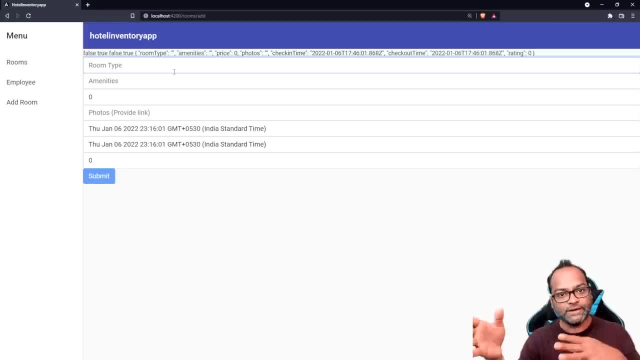 and it will be false. remember: valid invalid can change the state. i mean a invalid can change the state. i mean a invalid can change the state. i mean a form which was valid can become invalid. form which was valid can become invalid. form which was valid can become invalid. in case i remove some, 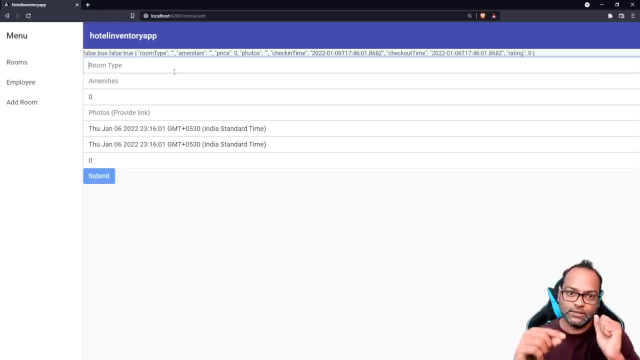 in case i remove some, in case i remove some values or delete some values from some values, or delete some values from some values or delete some values from some control, control, control. but a form which becomes pristine, but a form which becomes pristine, but a form which becomes pristine to dirty will never come back. 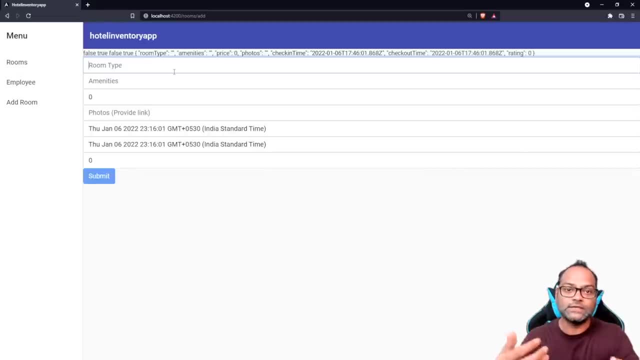 to dirty, will never come back to dirty, will never come back until until until, unless you reset it, until until until, unless you reset it, until until, until, until, unless you reset it. the thing is we are about to go ahead. the thing is we are about to go ahead. 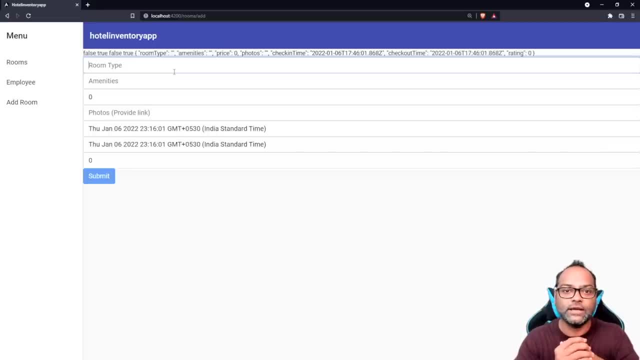 the thing is, we are about to go ahead and see how we can reset our form that's and see how we can reset our form that's and see how we can reset our form. that's why we are talking about dirty and uh, why we are talking about dirty and uh. 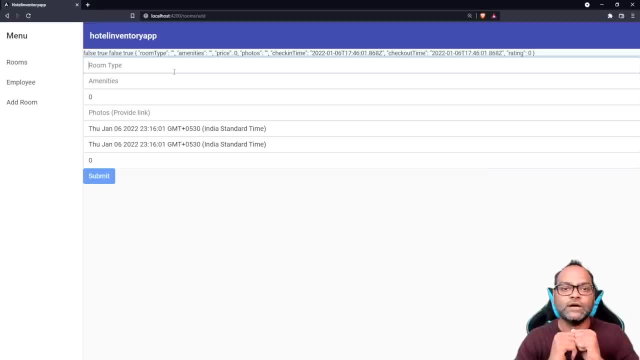 why we are talking about dirty and uh, pristine. so remember: pristine means pristine. so remember, pristine means pristine. so remember: pristine means frustrated. i have as a user. no one has frustrated. i have as a user, no one has frustrated. i have as a user. no one has actually touched anything, no one has. 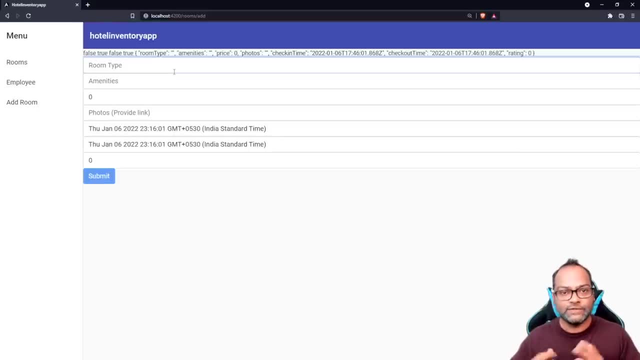 actually touched anything. no one has actually touched anything. no one has entered anything inside the controls, entered anything inside the controls, entered anything inside the controls, provided once you do interact with it, provided once you do interact with it, provided once you do interact with it, it becomes dirty. so these states are: 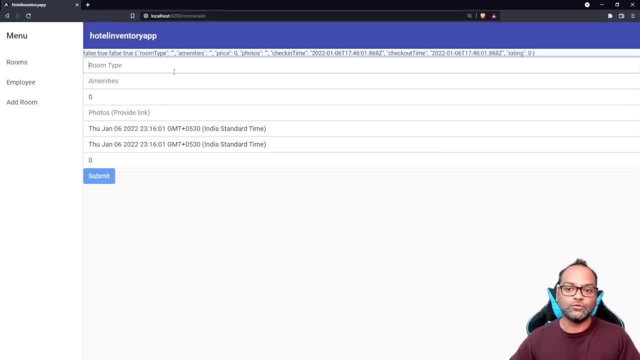 it becomes dirty, so these states are. it becomes dirty, so these states are actually really important. in case you actually really important, in case you actually really important, in case you want to understand, want to understand, want to understand, or you want to see if user has, or you want to see if user has. 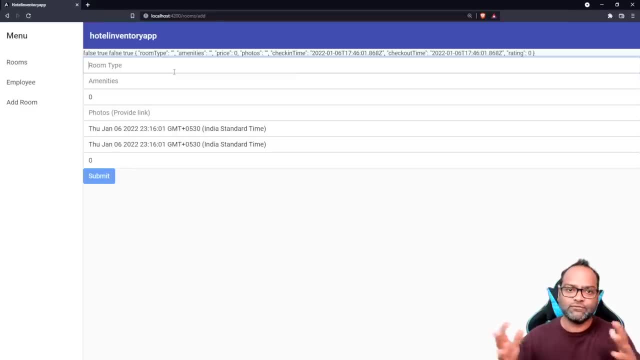 or you want to see if user has interacted with your form or not interacted with your form, or not interacted with your form or not. you may actually have, let's say, form. you may actually have, let's say, form. you may actually have, let's say, form where you want to collect some feedback. 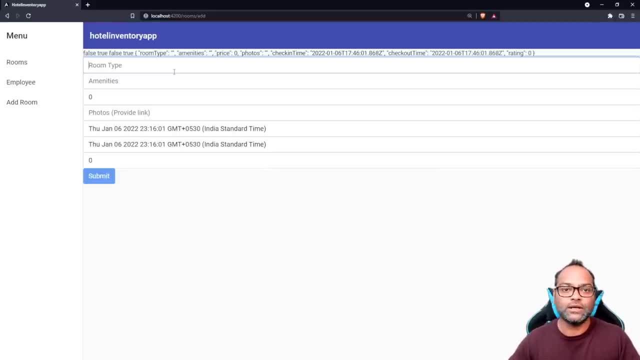 where you want to collect some feedback, where you want to collect some feedback, but you really want feedback, so sometime. but you really want feedback, so sometime. but you really want feedback, so sometime you may. so how you can do that, so based on this. so how you can do that, so based on this. 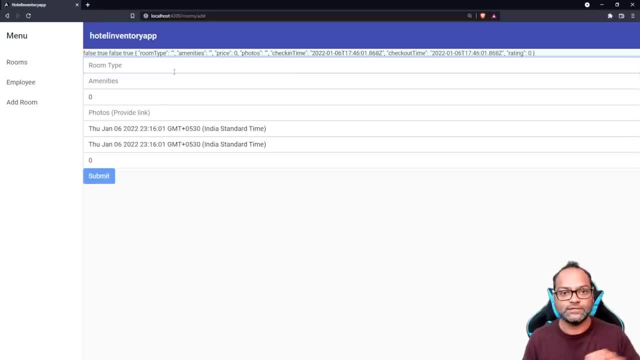 so how you can do that. so, based on this, state so if it's pristine or dirty, so state. so if it's pristine or dirty, so state. so if it's pristine or dirty, so let's say user entered something, and let's say user entered something and 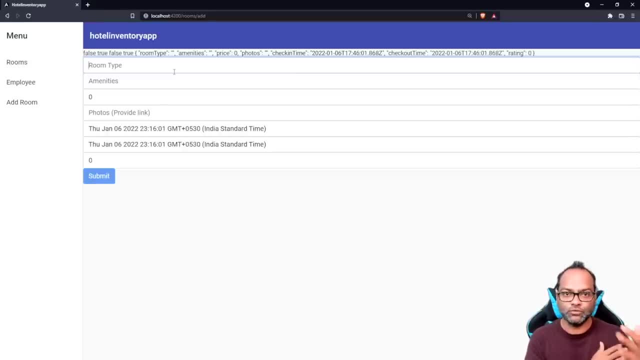 let's say, user entered something and then he decided to move out. you can just then he decided to move out. you can just then he decided to move out. you can just restrict him. okay, uh, you have some restrict him. okay, uh, you have some restrict him. okay, uh, you have some unsafe changes. or let's say, it is a 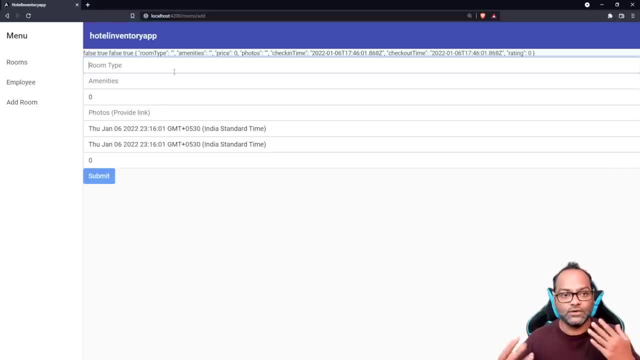 unsafe changes, or let's say it is a unsafe changes, or let's say it is a really important form right. you have really important form right. you have really important form right. you have stepper control, for example. in case you stepper control. for example, in case you stepper control. for example, in case you now, uh, as you understand, pristine and 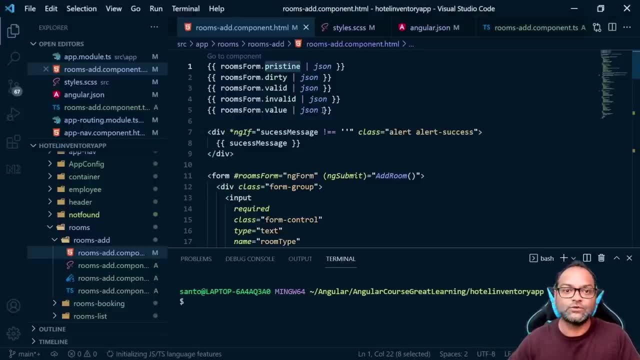 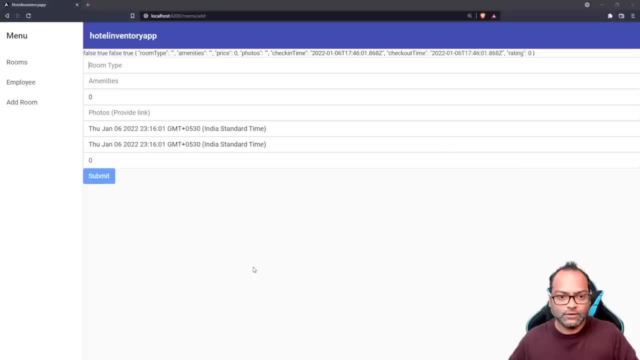 now, uh, as you understand, pristine. and now, uh, as you understand, pristine, and ready now let's move back. uh, sorry, so ready now let's move back. uh, sorry, so ready now let's move back. uh, sorry, so let's go ahead and talk about how to reset the form right. 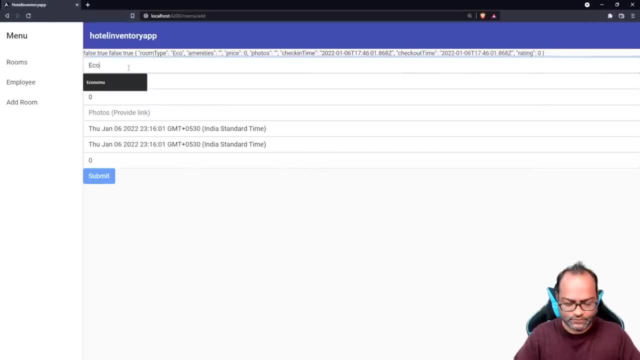 how to reset the form right. how to reset the form right. if you see this right now, uh, we have. if you see this right now, uh, we have. if you see this right now, uh, we have. let's say go on, let's say go on, let's say go on wi-fi. 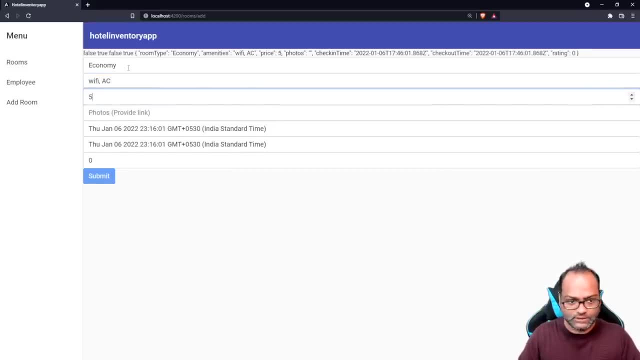 wi-fi, wi-fi, ac, ac, ac, and let's say this is 5000, this is, and let's say this is 5000, this is, and let's say this is 5000, this is anything, and, uh, you might be wondering anything and, uh, you might be wondering. 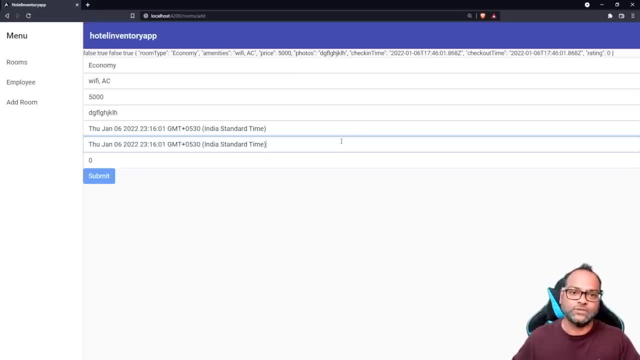 anything and, uh, you might be wondering why this is not date time? because, uh, the why this is not date time? because, uh, the why this is not date time? because, uh, the date time control is actually broken on. date time control is actually broken on. date time control is actually broken on. i think this is a chromium browser, so i 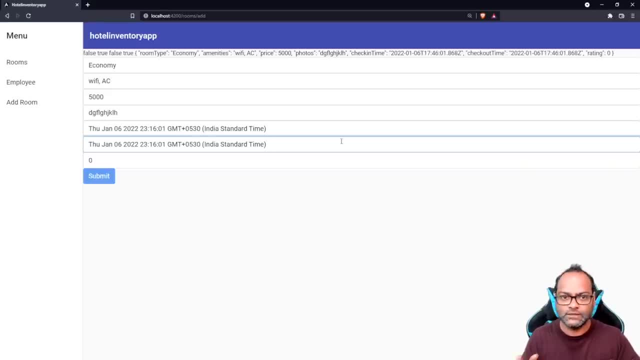 i think this is a chromium browser, so i i think this is a chromium browser, so i i'll replace this with. i'll replace this with. i'll replace this with material date picker, and we will do that: material date picker, and we will do that material date picker, and we will do that. we'll do that together, so just wait. 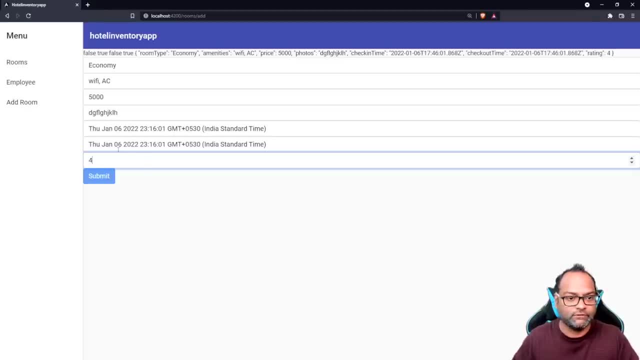 we'll do that together, so just wait. we'll do that together, so just wait. right now, it's it's uh the default date. right now, it's it's uh the default date. right now, it's it's uh the default date. right and then, right and then. 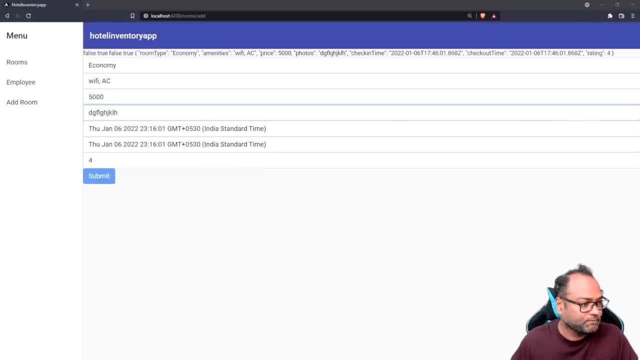 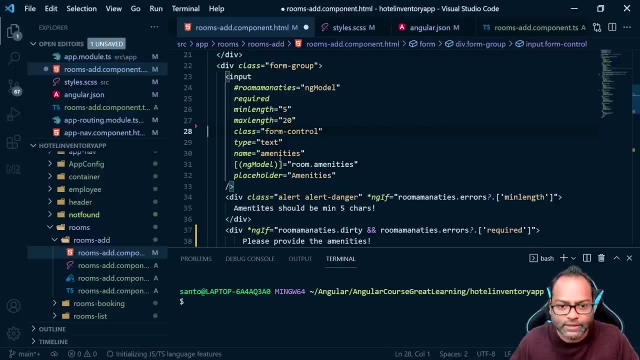 right, and then we can do, we can do, we can do. i have to remove one thing. i have to remove one thing. i have to remove one thing. remember: we added email, so we added pattern, so we added pattern, so we added pattern. yeah, yeah, yeah, let's remove the pattern so we can. 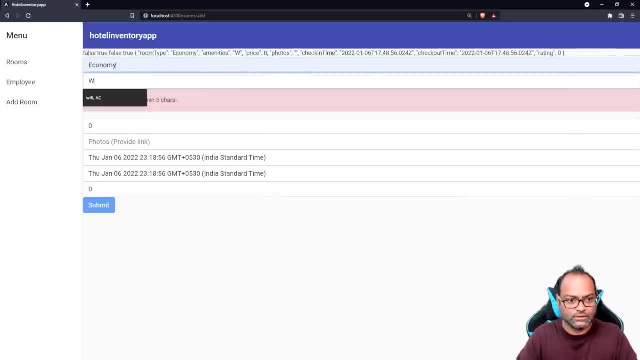 let's remove the pattern so we can. let's remove the pattern so we can actually go ahead and save the data. so actually go ahead and save the data, so actually go ahead and save the data. so we say, okay, this is economy, i think i. we say, okay, this is economy, i think i. 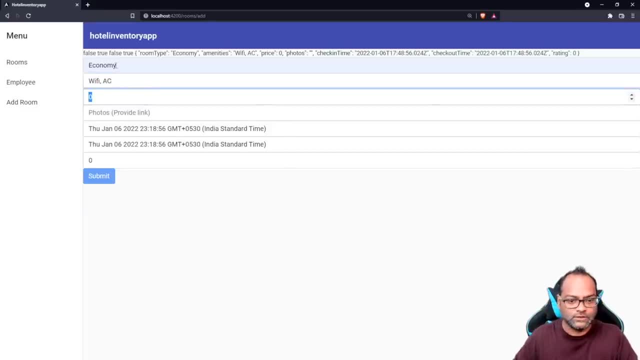 we say: okay, this is economy. i think i have have have five pipe and then ac, five pipe and then ac, five pipe and then ac, and let's say this is 5k, this is random. and let's say this is 5k, this is random. 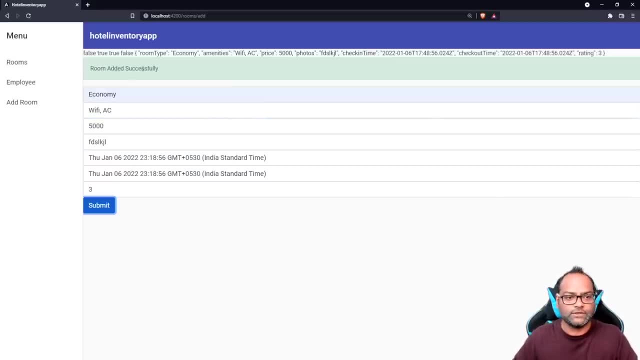 and let's say this is 5k, this is random data, and let's say this is three star data. and let's say this is three star data and let's say this is three star, let's say so. a room added successfully. let's say so, a room added successfully. 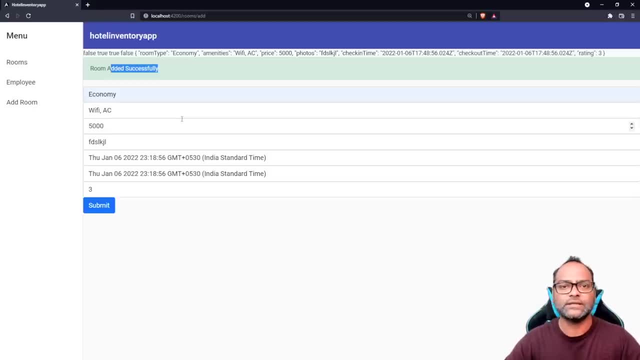 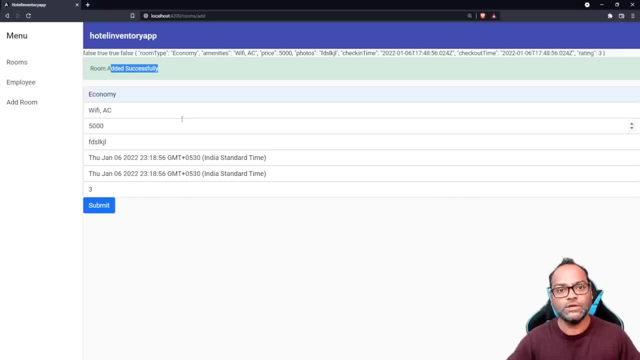 the data is still there. don't you think this is wrong? yes, it is wrong. i mean we. this is wrong. yes, it is wrong. i mean we. this is wrong. yes, it is wrong. i mean we should reset the form so i can, as a user, should reset the form so i can, as a user. 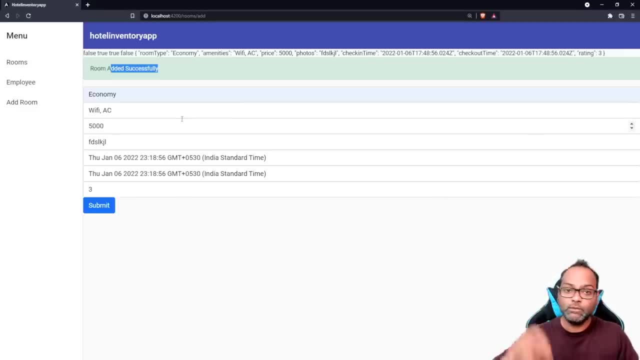 should reset the form so i can, as a user, i can enter new data right it. i can enter new data. right it. i can enter new data. right it may be possible. if you still show this may be possible. if you still show this may be possible. if you still show this data, the uh user may actually just. 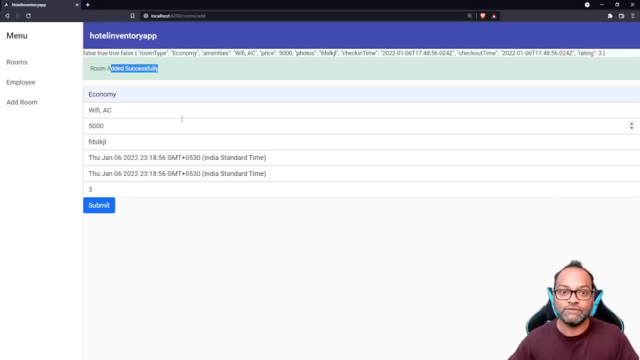 data. the uh user may actually just data. the uh user may actually just duplicate the data by by wondering, okay, duplicate the data by by wondering okay. duplicate the data by by wondering, okay, why this still data is still available, why this still data is still available, why this still data is still available here. so let's see how we can reset the. 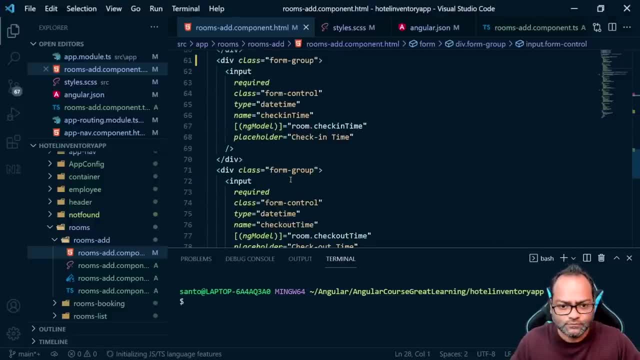 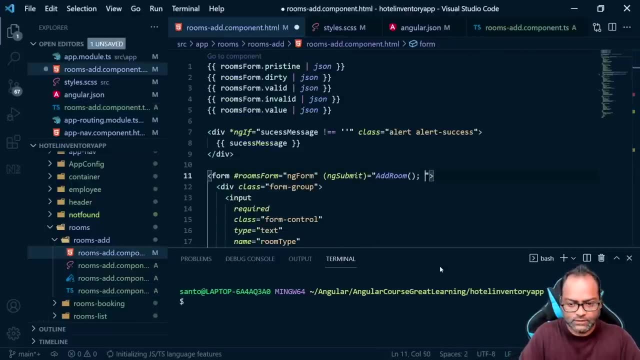 here. so let's see how we can reset the here. so let's see how we can reset the state reset the state of this form. so state reset the state of this form. so state reset the state of this form. so to do that, we can, we can. 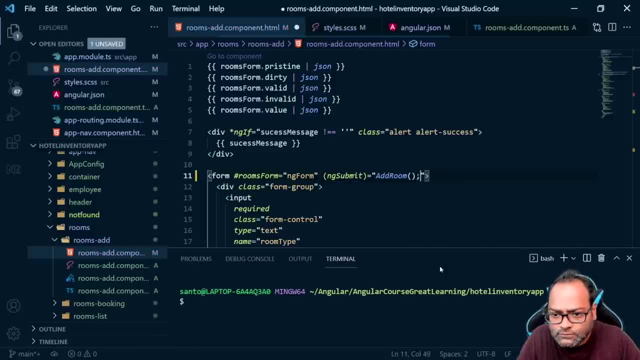 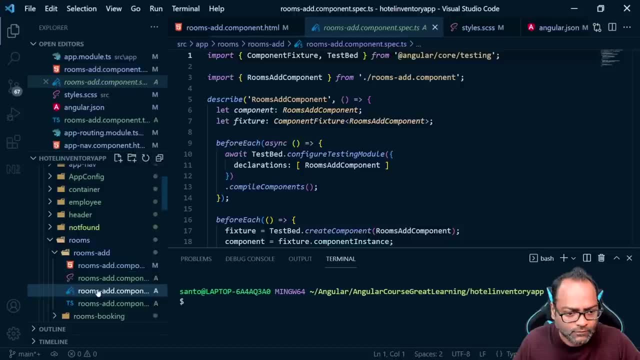 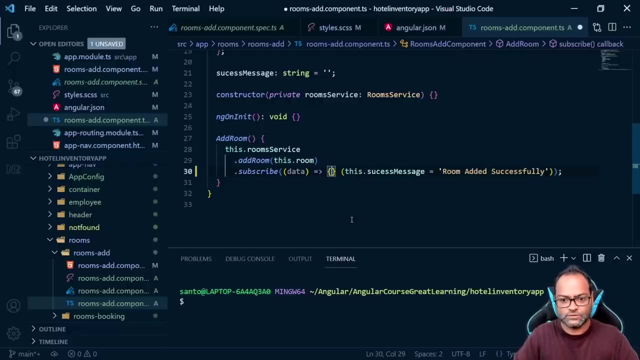 we can say here: let's go back, so i want to reset the state, let's go back, so i want to reset the state, let's go back. so i want to reset the state after the operation is completed, right so, after the operation is completed, right so. 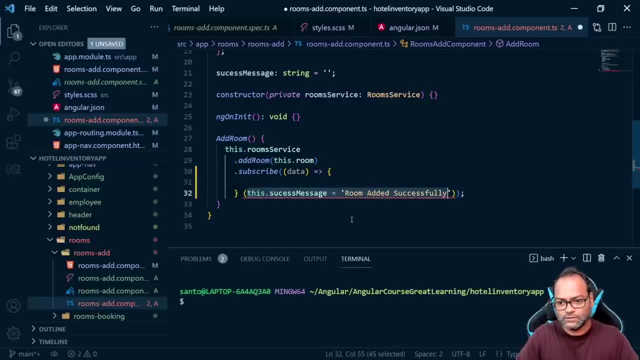 after the operation is completed: right, so i can do something like this here, so i, i can do something like this here, so i, i can do something like this here, so i can, let's, let's, let's just remove, and then, uh, we can get the access to this. 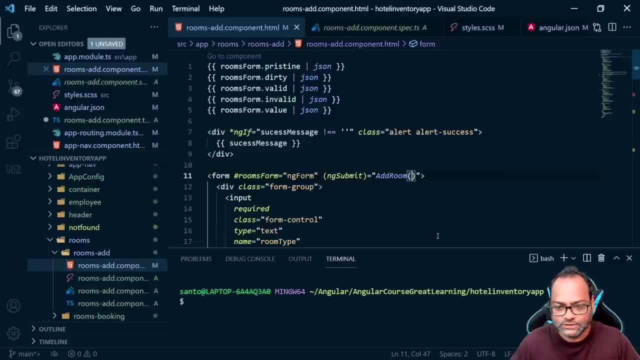 and then, uh, we can get the access to this. and then, uh, we can get the access to this. form control how we can do that. so we form control how we can do that. so we form control how we can do that, so we can actually pass, can actually pass. 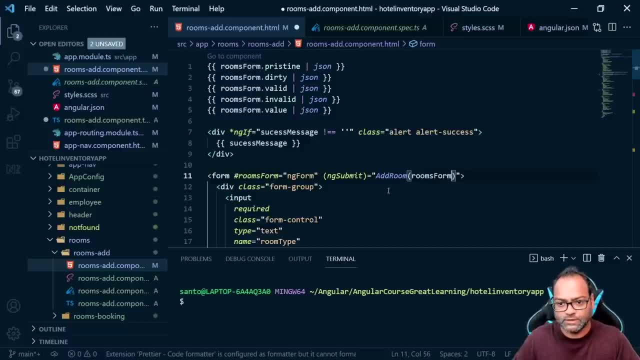 can actually pass this room's form, this room's form, this room's form as a variable here, as a variable here, as a variable, here and now, here we will get this room's. and now, here we will get this room's. and now, here we will get this room's form, which is, which will be type of ng. 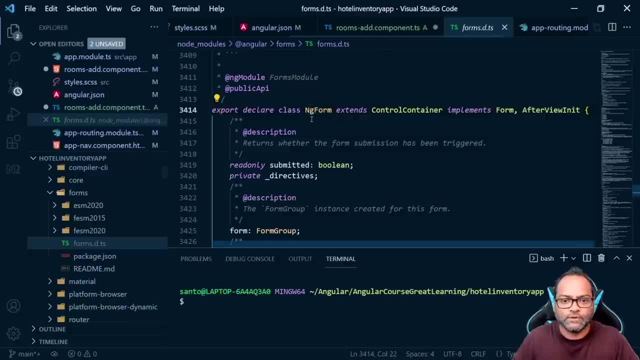 form, which is which will be type of ng form, which is which will be type of ng form, form form, and, and and let's see if i am. let's see if i am. let's see if i am accessing the current yeah control. accessing the current yeah control. 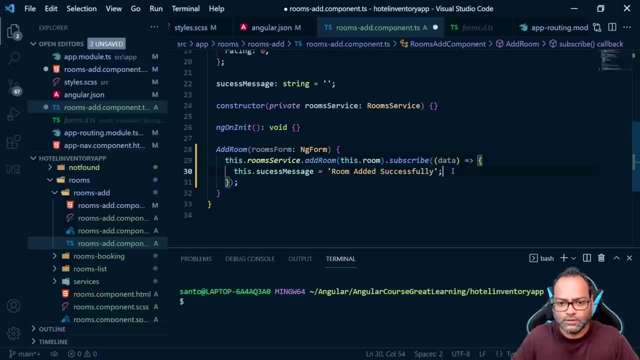 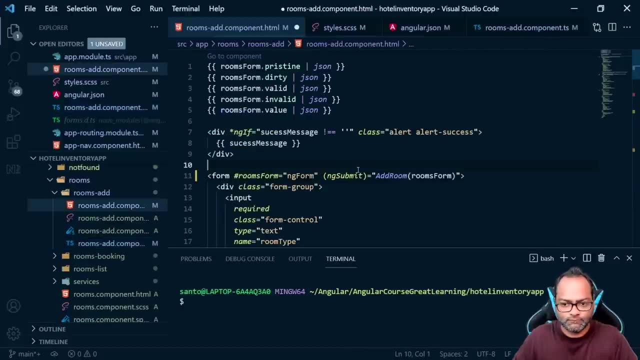 accessing the current: yeah, control container, yep container, yep container, yep. so after this i can say rooms form dot reset. after this i can say rooms form dot reset. after this i can say rooms form dot reset. so let's see how it behaves and let's say both. 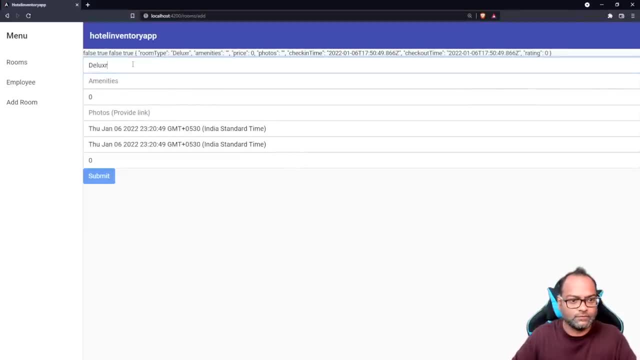 so i'll say: this is deluxe. so i'll say: this is deluxe, so i'll say: this is deluxe: amenities, amenities, amenities, high five, high five, high five. tv. you see, and then you see, and then you see, and then there's a six case, random data, four star. 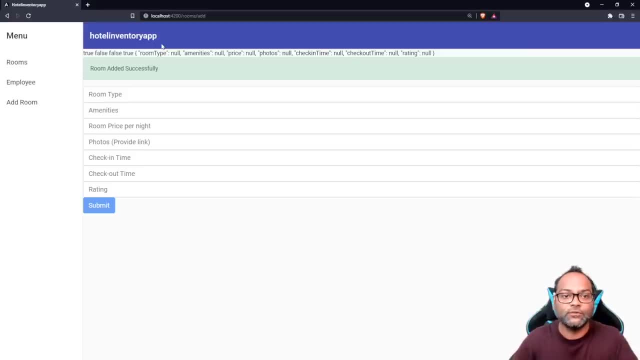 there's a six case random data- four star. there's a six case random data four star and save now you can see your room is and save now you can see your room is and save now you can see your room is added successfully and now. added successfully and now. 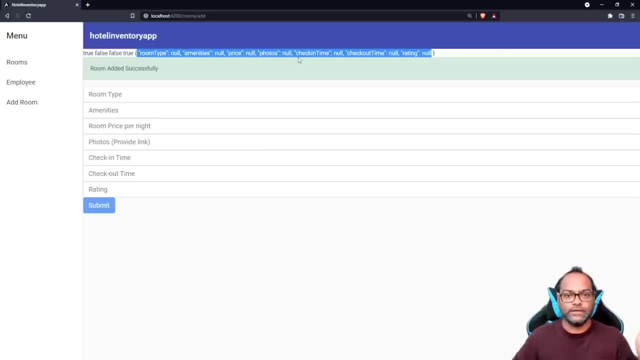 added successfully and now your entire data is actually resetted. your entire data is actually resetted. your entire data is actually resetted. right, so now we have a fresh state. you right, so now we have a fresh state. you right, so now we have a fresh state. you can see also: 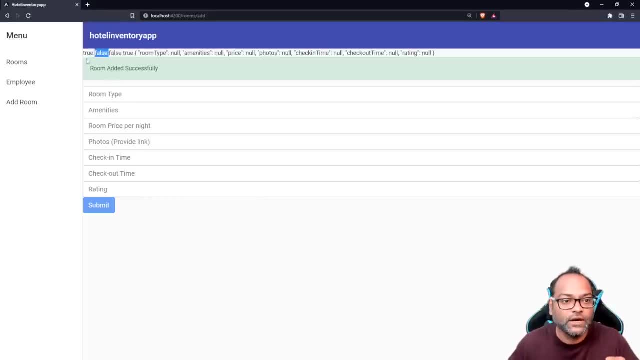 can see also. can see also the most important thing to understand. the most important thing to understand, the most important thing to understand: here is once you reset your form, here is once you reset your form. here is once you reset your form, pristine. that's why it became true. 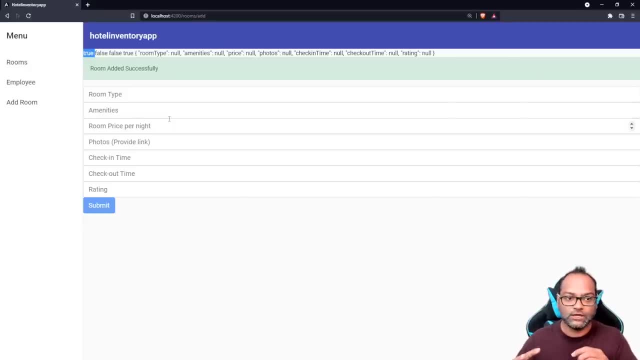 pristine. that's why it became true. pristine. that's why it became true. otherwise, it will never become true. so otherwise, it will never become true. so otherwise, it will never become true. so this is this is how you can actually. this is this is how you can actually. 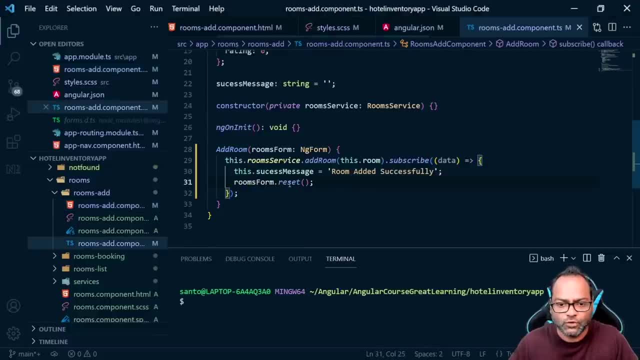 this is, this is how you can actually reset the state of form as well, reset the state of form as well, reset the state of form as well. and there are a few more methods. so you and there are a few more methods. so you and there are a few more methods, so you can also do. 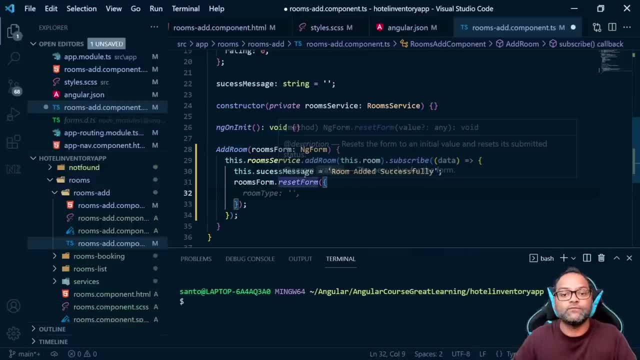 can also do, can also do reset form, and here you can actually pass reset form, and here you can actually pass reset form, and here you can actually pass the default data. so i can just do the default data, so i can just do the default data, so i can just do: uh, here i can just copy this and i can 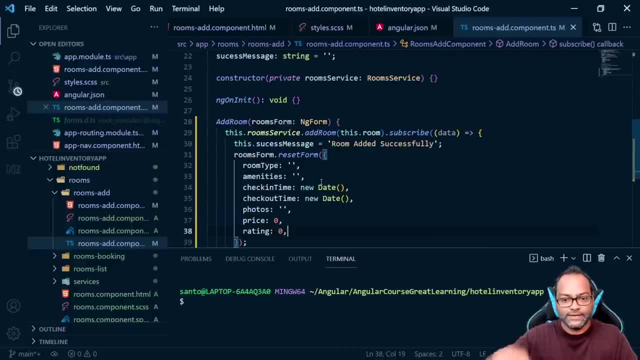 uh, here, i can just copy this and i can. uh, here, i can just copy this and i can say: okay, say okay, say okay, once you reset the form, just go ahead. and once you reset the form, just go ahead. and once you reset the form, just go ahead and treat this as default data. let's see. 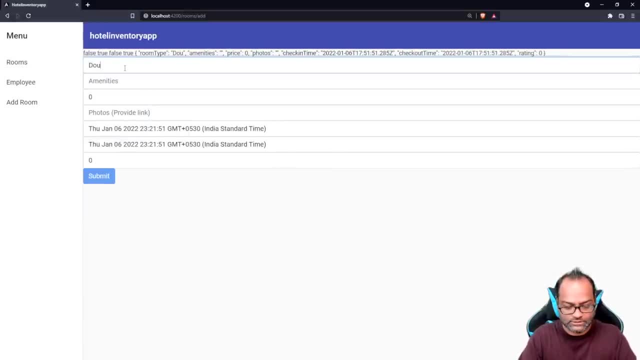 treat this as default data. let's see. treat this as default data. let's see, i'll say this is deluxe. i'll say this is deluxe. i'll say this is deluxe. or you can say this is, or you can say this is, or you can say this is double room amenities. 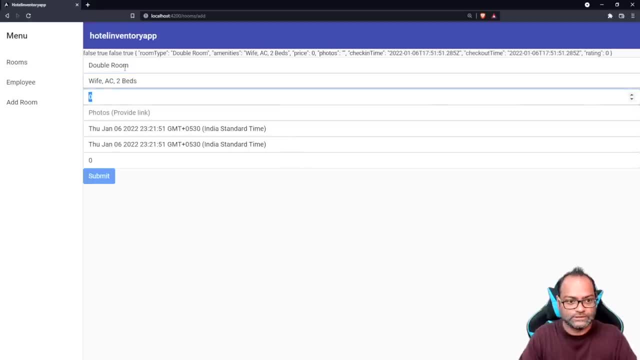 double room amenities. double room amenities: wi-fi ac, wi-fi ac, wi-fi ac- two beds, and let's say this is 5500, two beds. and let's say this is 5500, two beds. and let's say this is 5500 and let's say this is four star right. 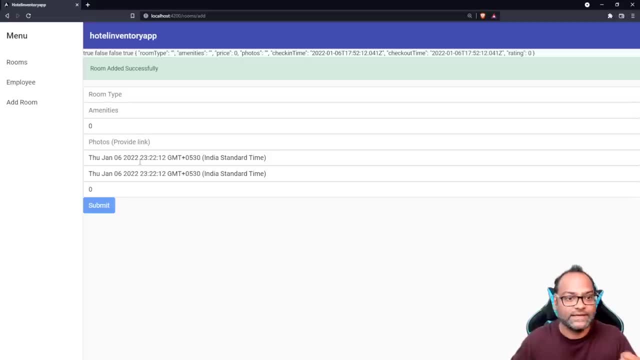 and let's say: this is four star right. and let's say this is four star right, submit. and now you have a reset state as submit, and now you have a reset state as submit, and now you have a reset state as well, of course, because you can see. 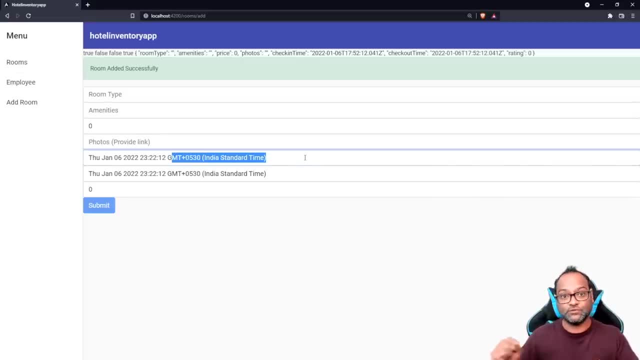 well, of course, because you can see. well, of course, because you can see, pristine became true and you have this pristine became true. and you have this pristine became true and you have this default data which you provided, so default data which you provided, so default data which you provided. so these are two methods which we can use. 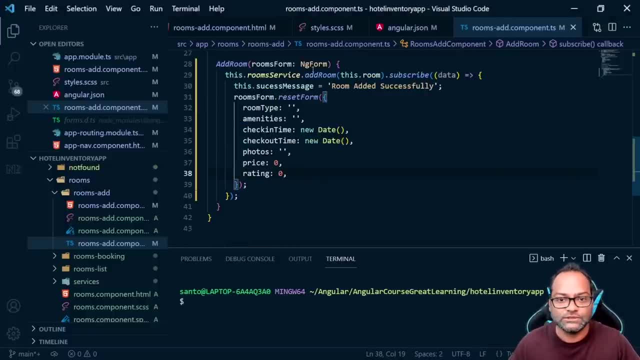 these are two methods which we can use. these are two methods which we can use to reset your forms using template. to reset your forms using template. to reset your forms using template driven form. so driven form, so driven form. so remember how we do this. so we are passing. 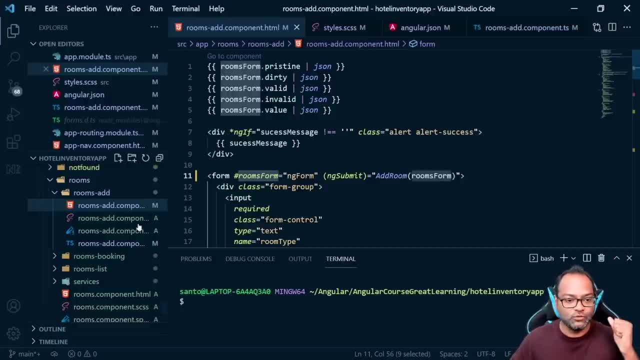 remember how we do this, so we are passing, remember how we do this, so we are passing this ng form, this ng form, this ng form as a reference to our type script file, as a reference to our type script file, as a reference to our type script file, and then we are saying, okay, this form is. 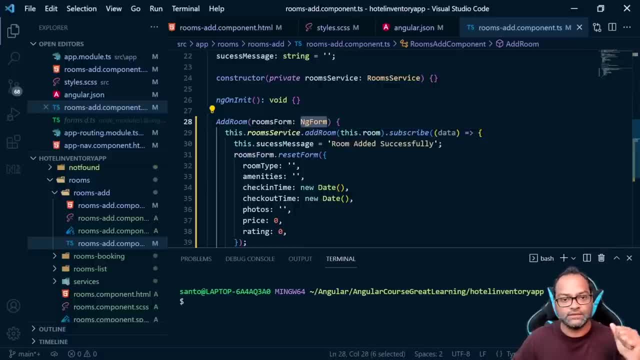 and then we are saying, okay, this form is. and then we are saying, okay, this form is actually actually actually type of ng form, because remember this, this type of ng form, because remember this, this type of ng form, because remember this, this ng form is like. ng form is like: 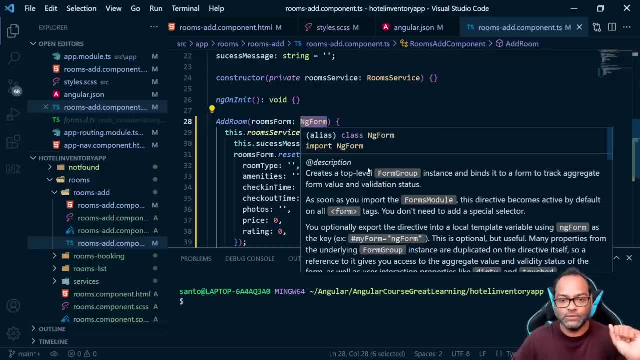 ng form is like uh extended, or you can say it's a top uh extended, or you can say it's a top uh extended, or you can say it's a top level form, group level form group level form group. which will be available. so under which? which will be available, so under which. 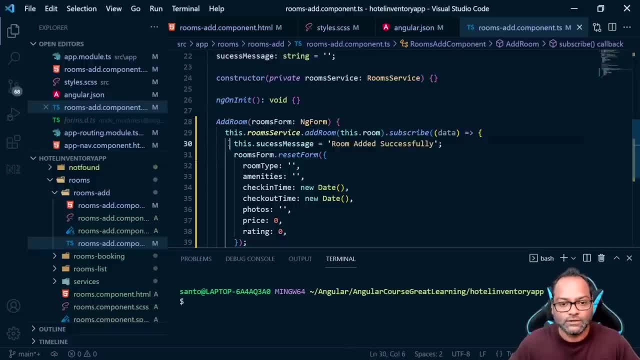 which will be available, so under which all the control will be available. all the control will be available, all the control will be available. and then, after you have added, and then after you have added, and then after you have added successfully, you can just go ahead and successfully, you can just go ahead and. 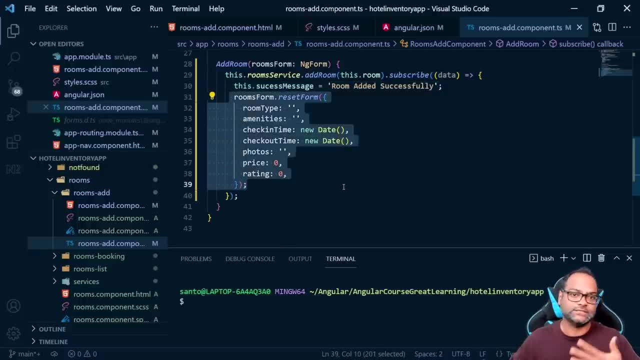 successfully. you can just go ahead and call the reset but reset form and call the reset but reset form and call the reset but reset form, and your state is reset now. your state is reset now. your state is reset now. so this is from: uh, this is how you can. 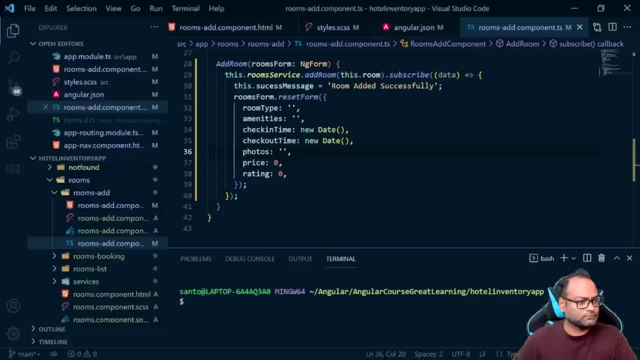 so this is from uh, this is how you can. so this is from uh, this is how you can actually actually actually handle the states and how you can reset, handle the states and how you can reset, handle the states and how you can reset your form. so next thing which we are going to talk, 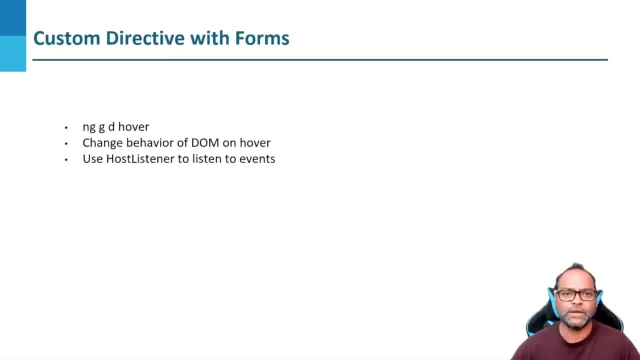 so next thing which we are going to talk, so next thing which we are going to talk about is custom directive with forms you about is custom directive with forms you about is custom directive with forms. you might be wondering where might be wondering, where might be wondering where the pipe part went. so pipe part will be. 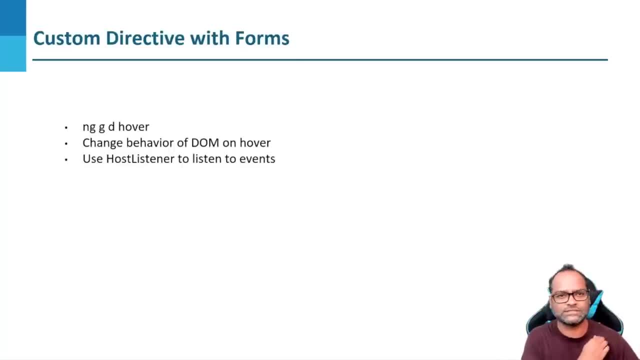 the pipe part went, so pipe part will be. the pipe part went, so pipe part will be actually covered in, actually covered in, actually covered in reactive form, because it's it's almost reactive form, because it's it's almost reactive form, because it's it's almost same. so i don't want to actually repeat. 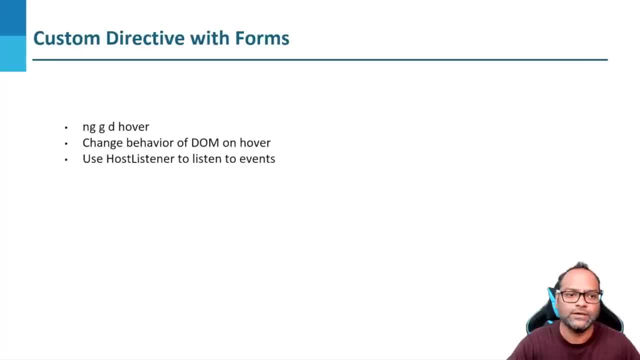 same. so i don't want to actually repeat same, so i don't want to actually repeat it again. it again, it again. so that's why we moved it there, and so that's why we moved it there, and so that's why we moved it there. and right now let's see how we can actually 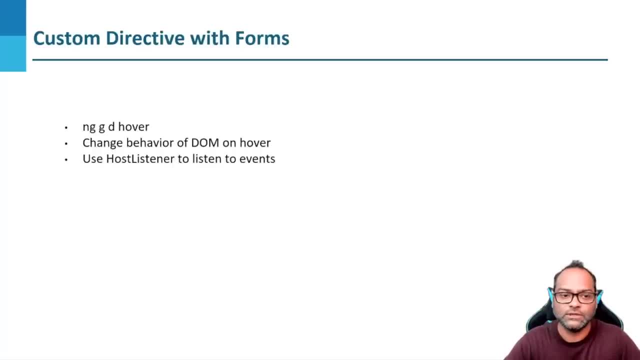 right now, let's see how we can actually right now, let's see how we can actually add a custom directive uh with forms, and add a custom directive uh with forms, and add a custom directive uh with forms. and what we are trying to do is we will be. 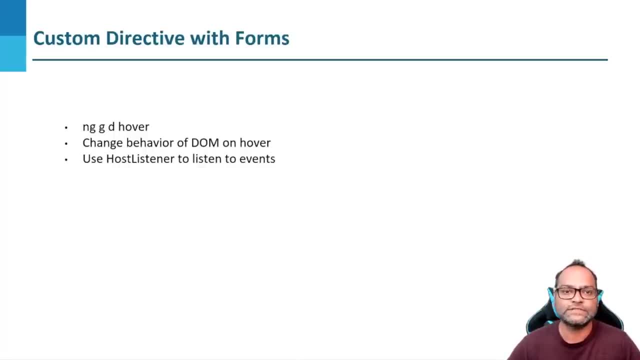 what we are trying to do is we will be. what we are trying to do is we will be: uh, uh, uh. we'll be creating a directive which can. we'll be creating a directive which can. we'll be creating a directive which can modify the behavior of an element. 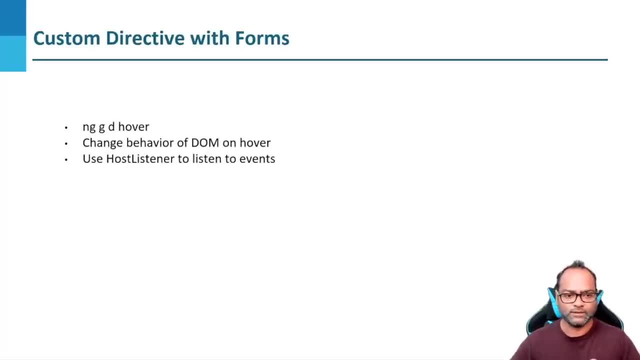 modify the behavior of an element. modify the behavior of an element. so what are the use cases? so uh, let's. so. what are the use cases? so uh, let's. so what are the use cases? so uh, let's see, see, see. uh, let's, let's see that right, so we will. 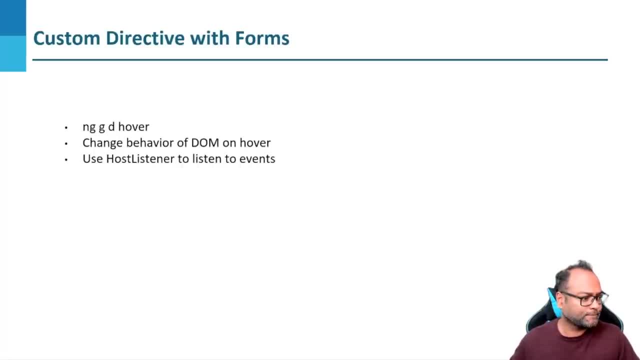 uh, let's, let's see that right, so we will. uh, let's, let's see that right, so we will talk about them. so, for this, what we are going to do is as so. for this, what we are going to do is as so. for this, what we are going to do is, as we are going to need a login form in: 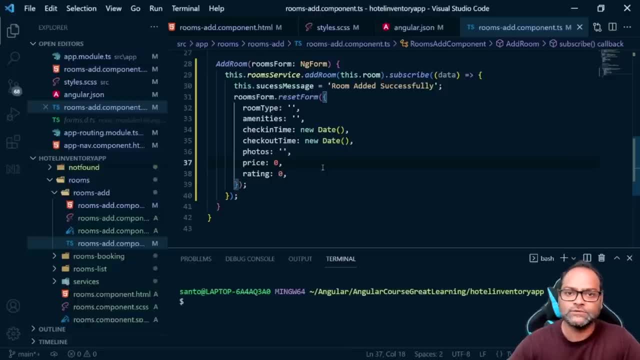 we are going to need a login form in. we are going to need a login form in future. we will create another form i we future, we will create another form i we future, we will create another form i. we will not touch this form as of now. we'll. 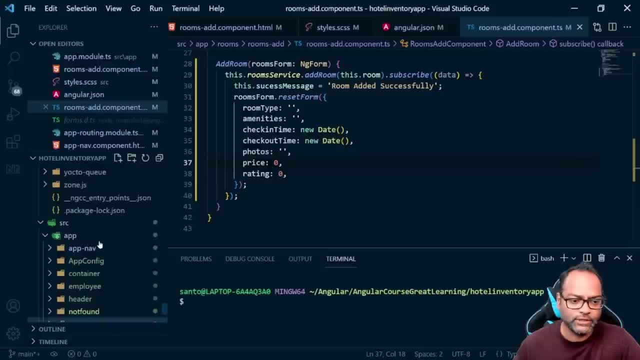 will not touch this form as of now. we'll will not touch this form as of now. we'll keep it as it is and let's create. keep it as it is and let's create. keep it as it is and let's create another component. uh, we will call it as. 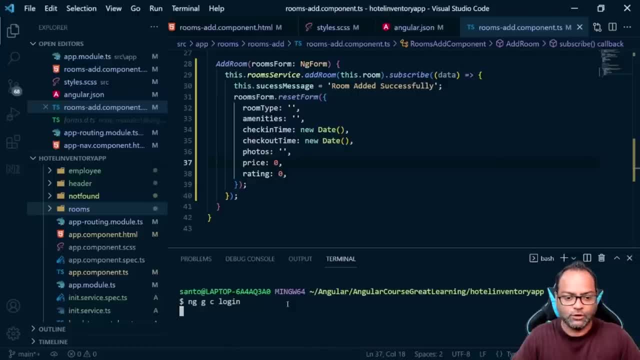 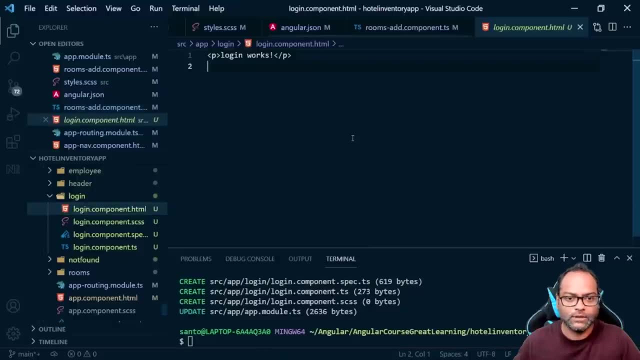 another component. uh, we will call it as another component. uh, we will call it as login component. so i'll say nggc login component, so i'll say nggc login, and we will be using template driven and we will be using template driven and we will be using template driven forms, and so let's go ahead and do that. 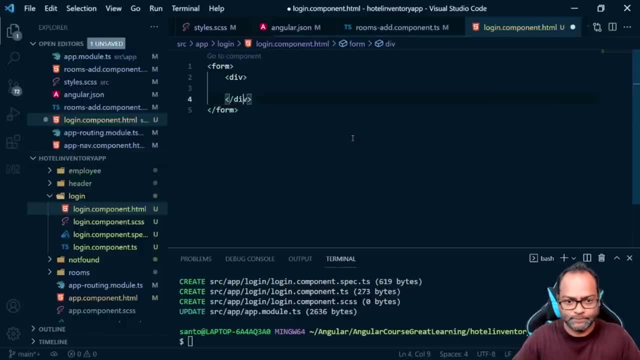 forms and so let's go ahead and do that. forms and so let's go ahead and do that. so it's a form, so it's a form, so it's a form, uh, div, and it's a class, and it's a class, and it's a class form. 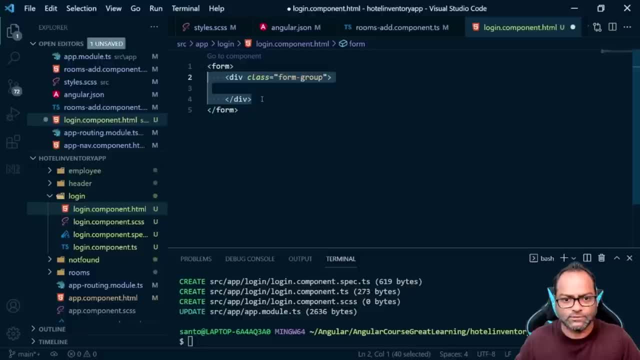 form form group. so i think form group is not group. so i think form group is not group. so i think form group is not working because of some conflicts with working, because of some conflicts with working, because of some conflicts with angular material, angular material, angular material. so let's see, 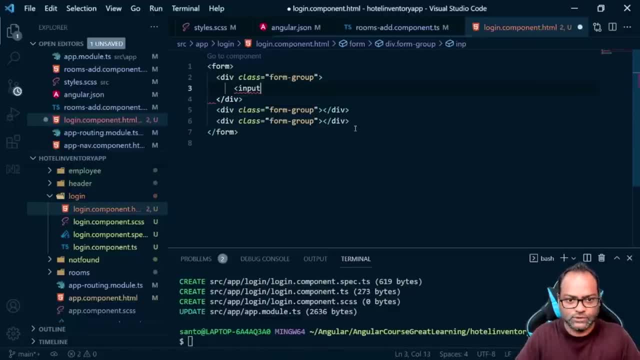 and we and we and we will and we will and we will add some controls. so this is input: add some controls. so this is input: add some controls. so this is input. type is text form: control, name ng model and i'll. text form control: name ng model and i'll. 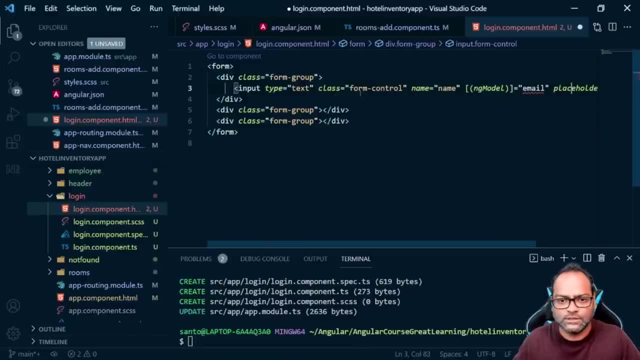 text form, control name, ng model, and i'll say say say this is email, let's this is email, let's this is email, let's say type is also email, because we are say type is also email, because we are say type is also email because we are going to treat. 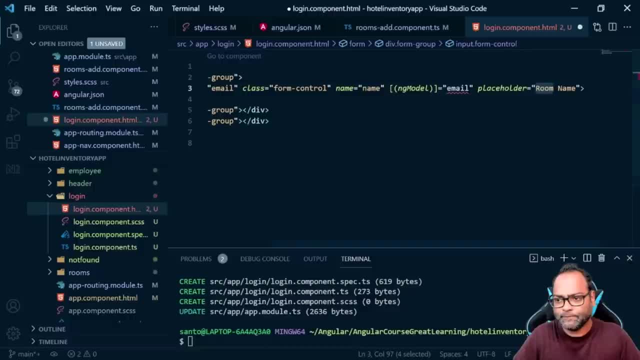 going to treat, going to treat uh username as email. i mean, provide, provide, provide your user, your user, your user. so, uh, we are not going to implement any. so, uh, we are not going to implement any. so, uh, we are not going to implement any api for this. we will actually. 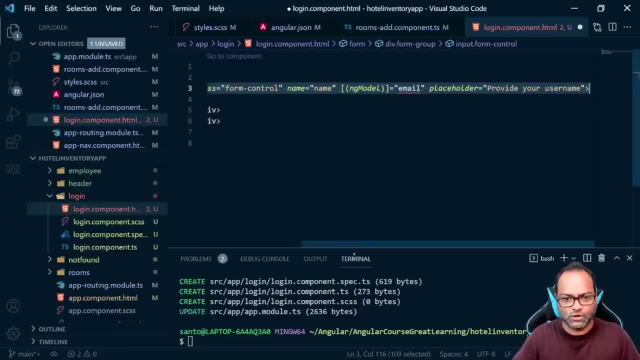 api for this. we will actually api for this. we will actually just mock and that's it. so we'll just just mock and that's it. so we'll just just mock and that's it. so we'll just mock this entire service with some dummy. mock this entire service with some dummy. 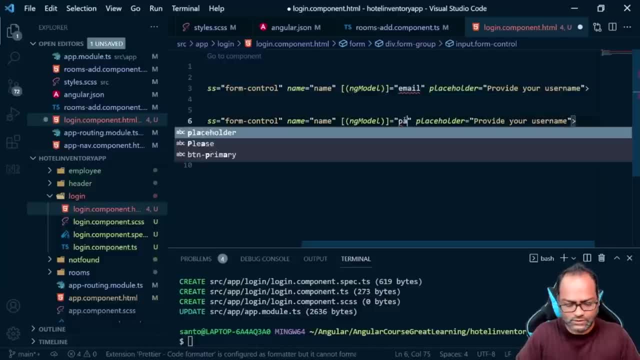 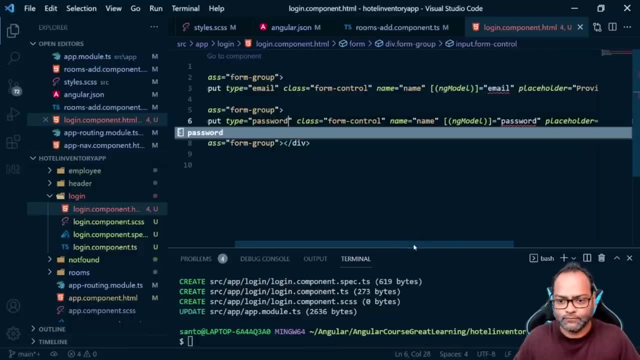 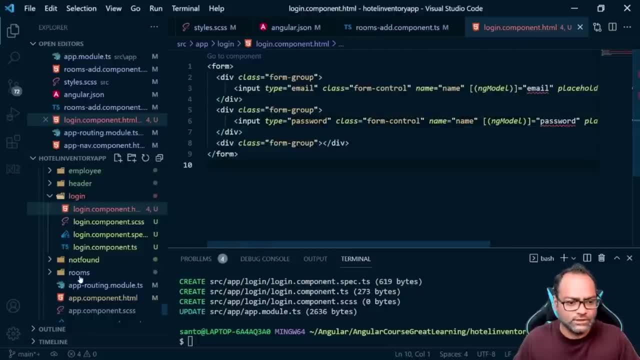 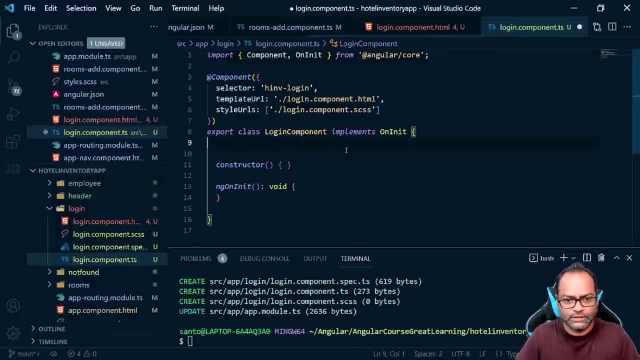 to create the model. let's go ahead and do that, do that, do that. so i'm going to create, so i'm going to create, so i'm going to create. uh, this is user name which is type of. uh, this is user name which is type of. 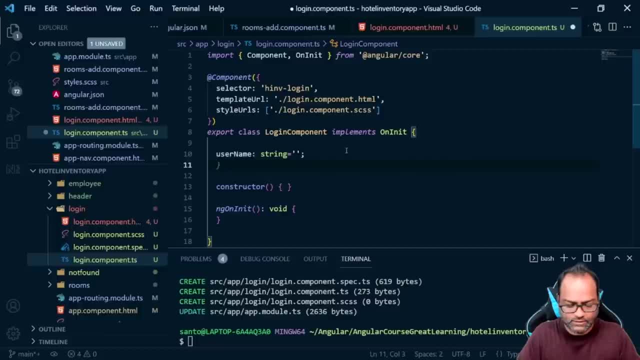 uh, this is user name, which is type of string: string, string. this equals to blank, this equals to blank, this equals to blank, and this will be password and this will be password and this will be password, which is again type of string. uh, let's. which is again type of string: uh, let's. 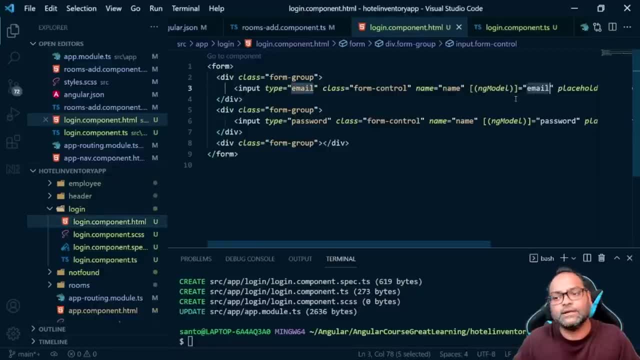 which is again type of string: uh, let's call this as email. so call this as email, so call this as email. so, because we have already, uh, yeah, we have. because we have already, uh, yeah, we have. because we have already, uh, yeah, we have used it as email, so let's do that and 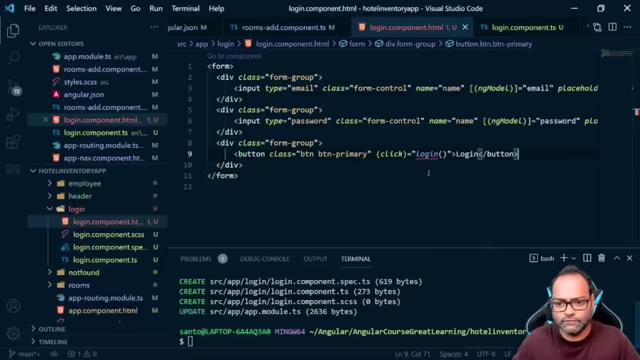 used it as email, so let's do that. and used it as email, so let's do that. and then we need a button, uh, so button. and then we need a button, uh, so button. and then we need a button, uh, so button. and we will, we will. 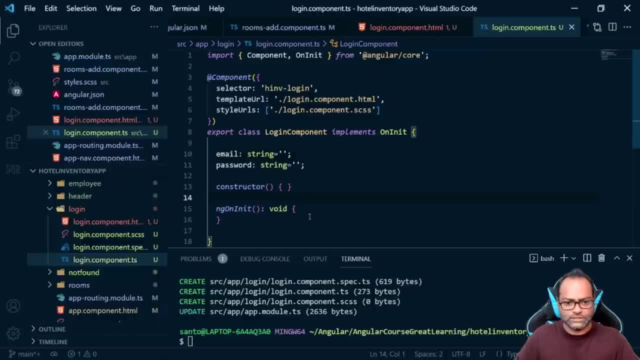 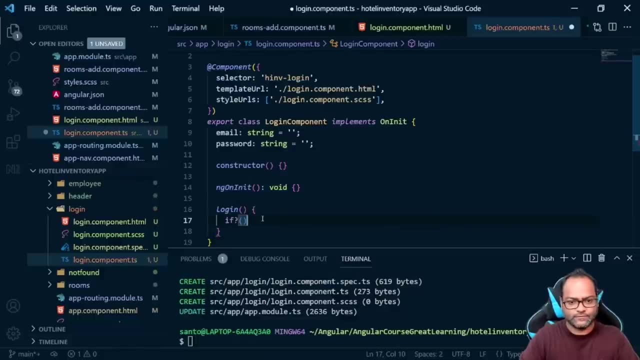 we will create a login button, create a login button, create a login button. so let's go ahead and write some logic. so let's go ahead and write some logic. so let's go ahead and write some logic here, here, here, login, and we'll say if this dot. 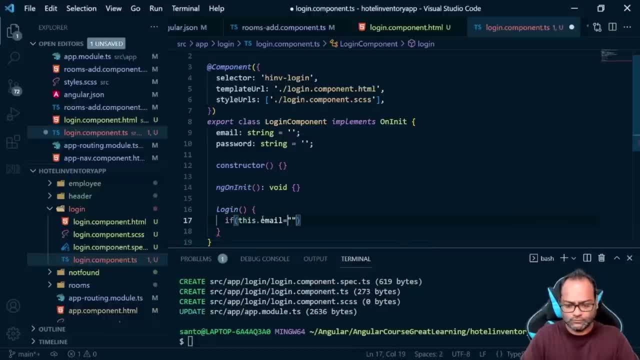 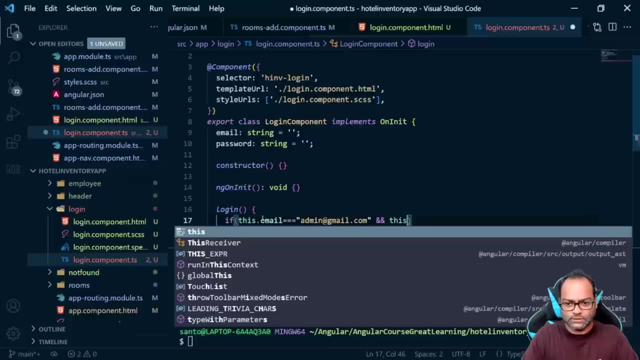 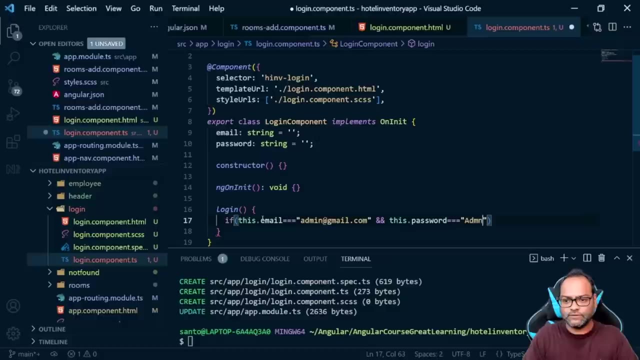 this dot. this dot email. email email is equals to admin. admin. admin at gmailcom, at gmailcom, at gmailcom, and, and, and this, this, this dot password, dot password. this equals to this dot password. this equals to this dot password. this equals to the best password in the world: admin admin. 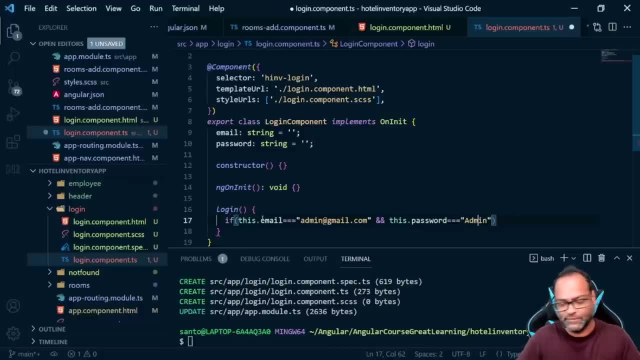 the best password in the world: admin: admin. the best password in the world: admin: admin. right so, right so, right. so username and password is admin. username and password is admin. username and password is admin. and let's see, and let's see, and let's see. and after this we have to go ahead and 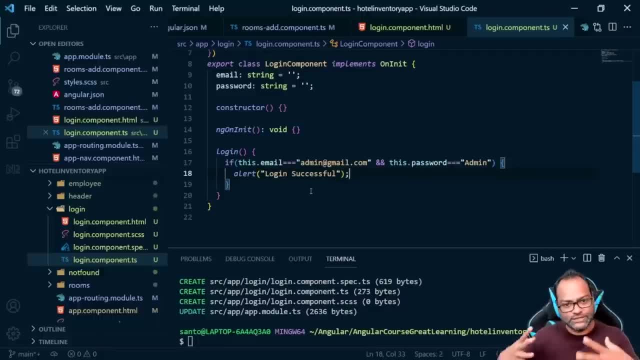 and after this, we have to go ahead, and, and after this, we have to go ahead. and let's- uh, right now, use an alert. let's- uh, right now, use an alert. let's- uh, right now, use an alert. and we have to actually go ahead, and, and we have to actually go ahead and. 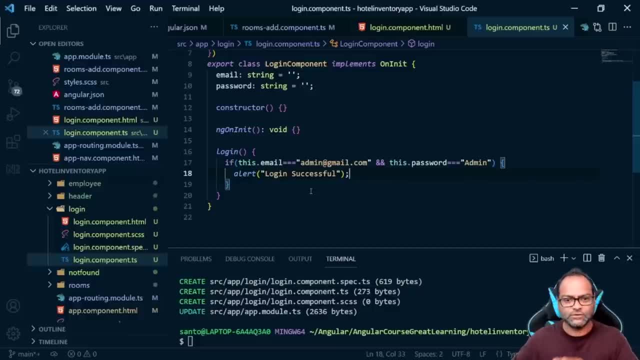 and we have to actually go ahead and implement this uh with some other, implement this uh with some other, implement this uh with some other. functionality of routing: we will come. functionality of routing, we will come. functionality of routing. we will come back to that later. right now, let's just 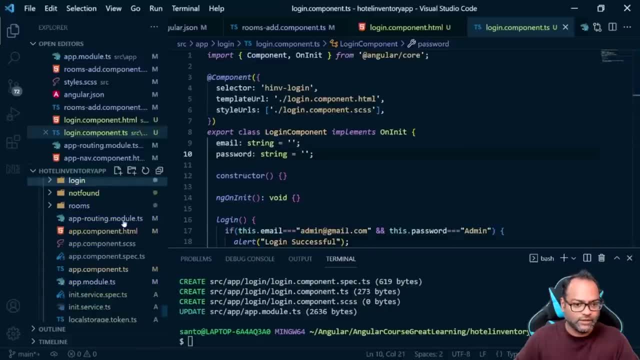 back to that later. right now, let's just back to that later. right now. let's just do this, do this, do this and here and here and here- uh, we will add route, uh, we will add route. uh, we will add route, we will redirect, we will redirect. 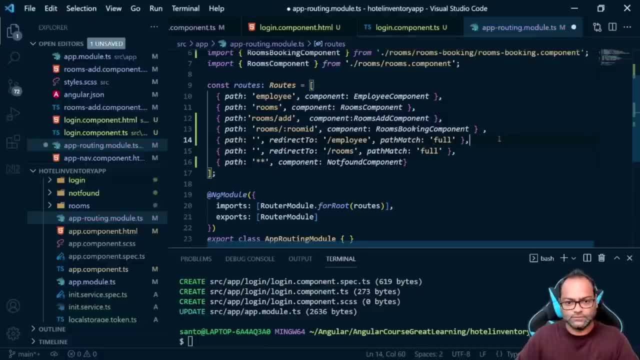 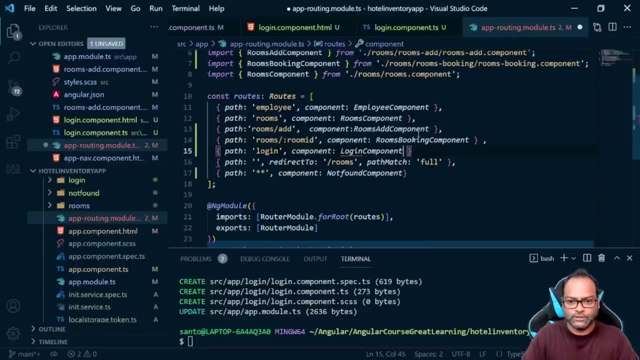 we will redirect. let's say: this is path, so the path is so. the path is so the path is login, login, login and component is login, component is login, component is login component. and now here we will redirect. and now here we will redirect. and now here we will redirect the users to login. 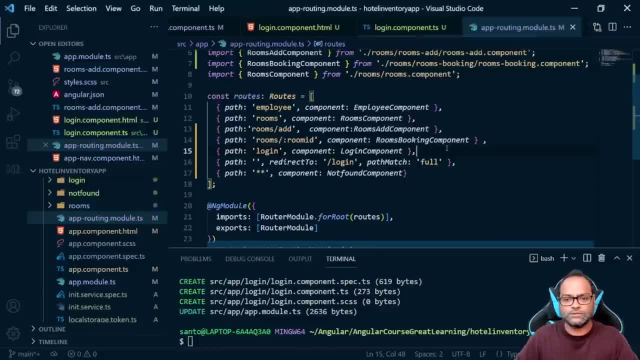 the users to login. the users to login. so we added a new component and let's so we added a new component and let's, so we added a new component and let's add a comma here. so add a comma here. so add a comma here. so, yeah, it's perfect. so we added a component. 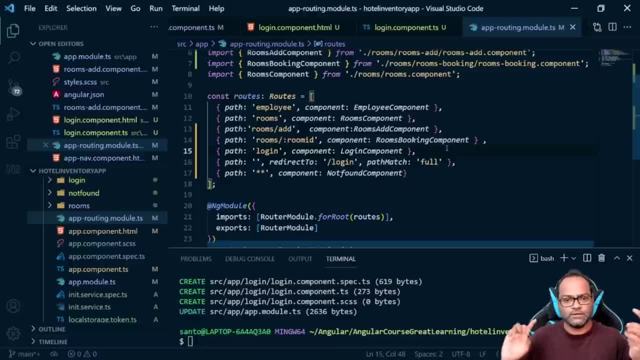 yeah, it's perfect, so we added a component. yeah, it's perfect, so we added a component. login component: we created a form login component. we created a form login component. we created a form for login and we now change the route. so, for login, and we now change the route. so. 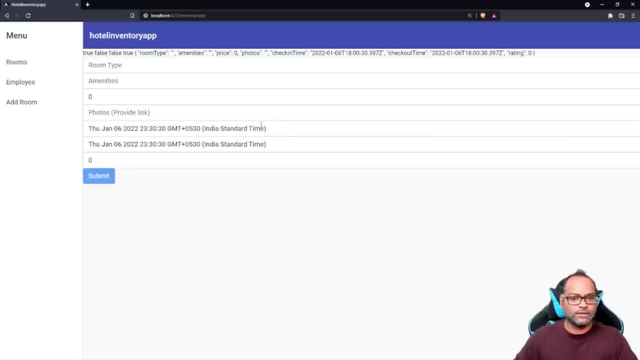 for login and we now change the route. so, by default, it will go to login. by default, it will go to login. by default, it will go to login. let's see, so, i'll, let's see, so, i'll, let's see, so i'll remove this, remove this. 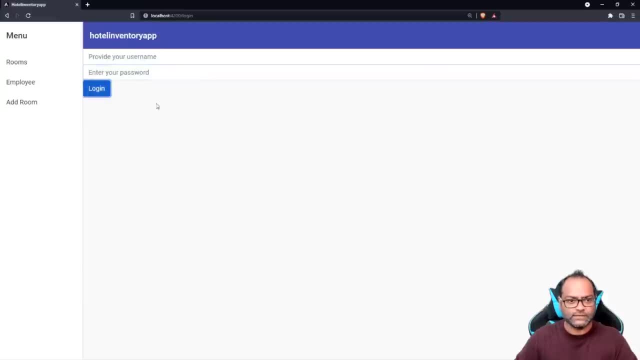 remove this. and here we go right, so provide username. and here we go right, so provide username. and here we go right, so provide username and password and password and password. and this login button, so right now of, and this login button, so right now of, and this login button, so right now. of course, the admin and password does not. 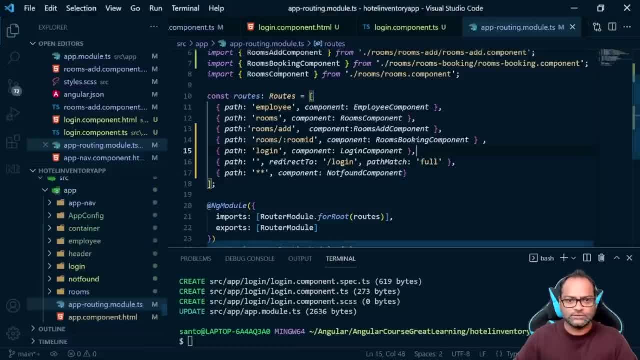 course the admin and password does not course. the admin and password does not match, so it will not show you another match. so it will not show you another match. so it will not show you another. but let's try that out. but let's try that out. but let's try that out. of course we wrote some logic, so let's. 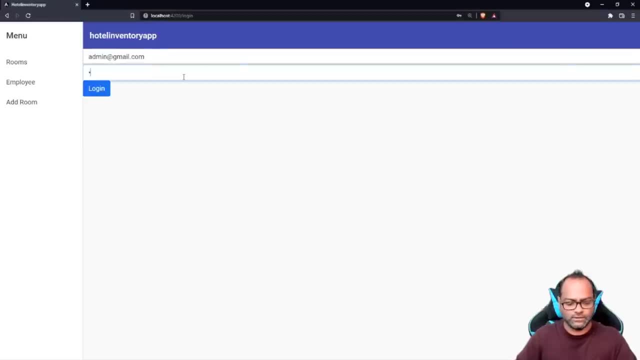 of course we wrote some logic, so let's. of course we wrote some logic, so let's verify. verify. verify: admin gmailcom and admin gmailcom and admin gmailcom and password is admin and yep login password is admin and yep login password is admin and yep login successful. 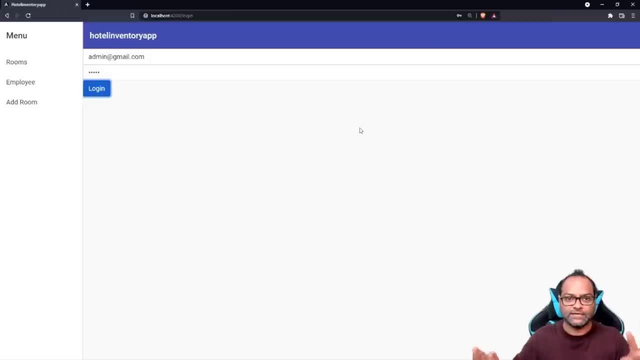 successful, successful hooray. we created our login page right. hooray, we created our login page right hooray, we created our login page right. i mean, of course you can design it in a. i mean, of course you can design it in a. i mean, of course you can design it in a better way. i'm not that great into a. 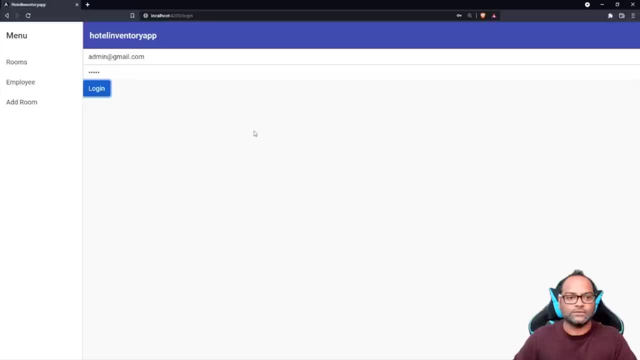 better way. i'm not that great into a better way, i'm not that great into a great using css, but yeah, i mean you can great using css. but yeah, i mean you can great using css. but yeah, i mean you can uh, uh, uh, you, you can design as per. 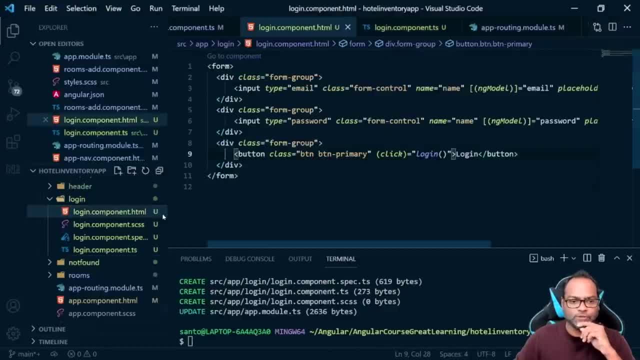 you. you can design as per you. you can design as per your knowledge, your knowledge, your knowledge. so, here, uh, what we are going to do, is we? so here, uh, what we are going to do, is we? so, here, uh, what we are going to do is we are going to create. 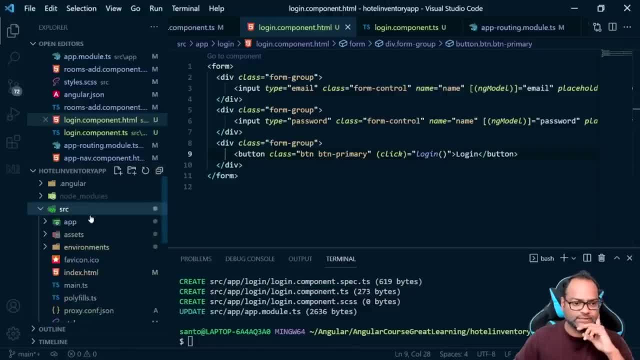 are going to create are going to create. we saw inbuilt directives so far. we saw inbuilt directives so far. we saw inbuilt directives so far. so let's go and create a new component. so let's go and create a new component. so let's go and create a new component. i'll just 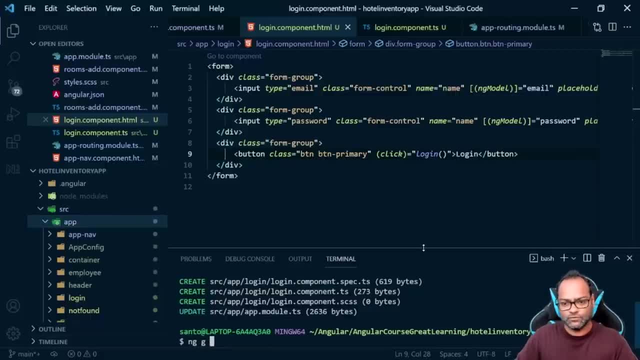 i'll just, i'll just try and say ngg to create a new. try and say ngg to create a new. try and say ngg to create a new directive. you can say ngg directive, you can say ngg directive, you can say ngg directive d and we'll call this component. 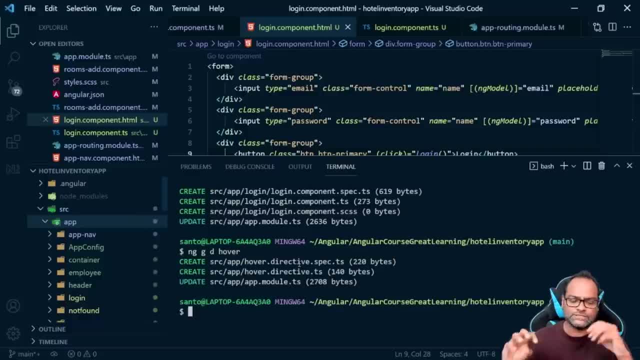 directive d, and we'll call this component directive d and we'll call this component directive as hovered. so directive as hovered, so directive as hovered. so what we want to achieve is whenever we. what we want to achieve is whenever we. what we want to achieve is whenever we hover above this particular elements. it 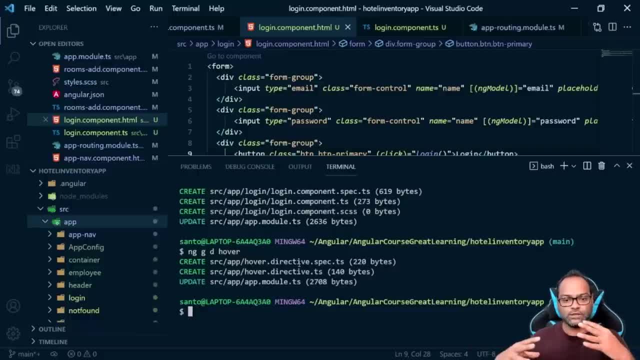 hover above this particular elements. it hover above this particular elements. it may change the background color, right, so may change the background color right, so may change the background color right. so, a minimal example to give you a real, a minimal example, to give you a real, a minimal example, to give you a real time. 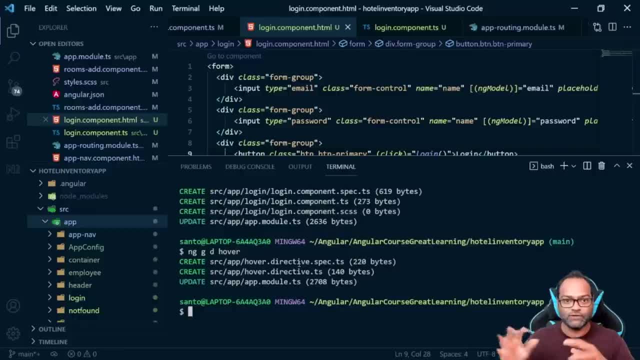 time time field of how you can actually write, a field of how you can actually write, a field of how you can actually write a directive which can modify directive, which can modify directive, which can modify your element of course in real-time, your element of course in real-time. 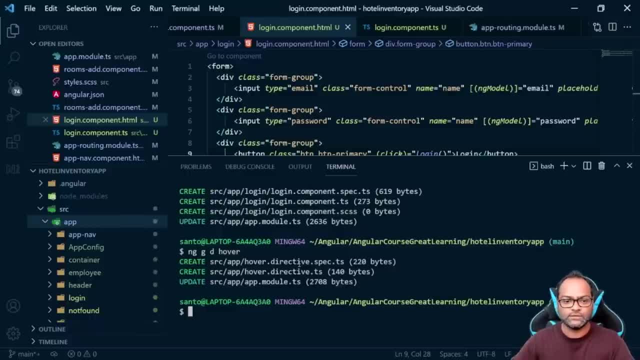 your element, of course, in real-time application. you will get more application. you will get more application. you will get more advanced use cases, but uh, advanced use cases, but uh, advanced use cases, but uh, i mean, this is, this is one of the. i mean, this is, this is one of the. 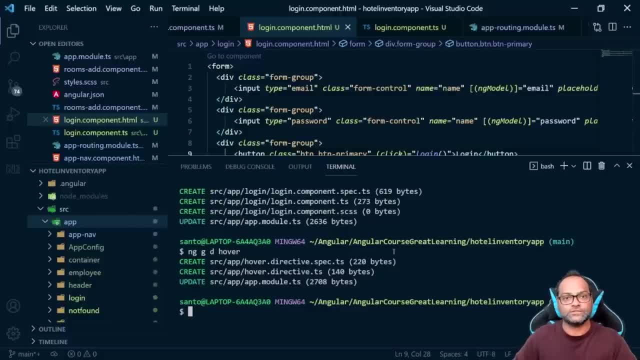 i mean, this is, this is one of the examples, which examples, which examples which can help you when you will plan to, can help you when you will plan to, can help you when you will plan to actually write some of the directives, actually write some of the directives. 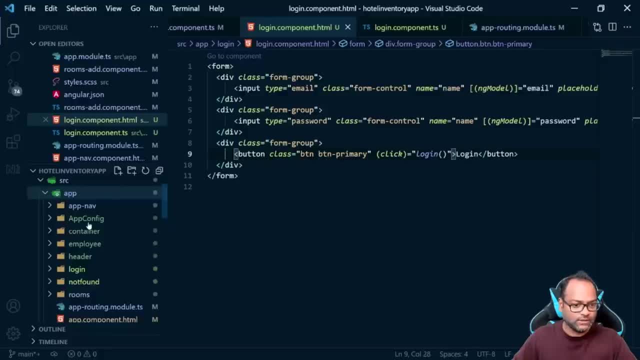 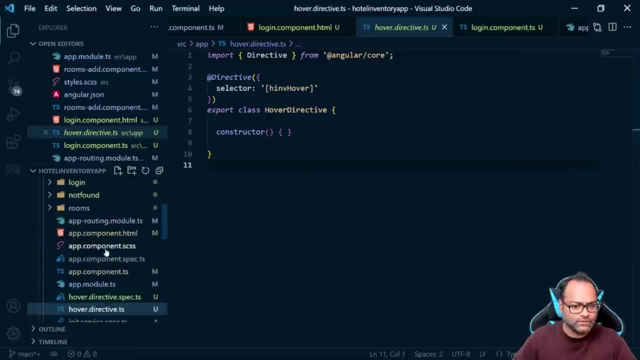 actually write some of the directives like this, like this, like this, so not, uh, done. now we can go to whole directive here. so let's go ahead. whole directive here. so let's go ahead. whole directive here. so let's go ahead and create a folder. so, and create a folder so. 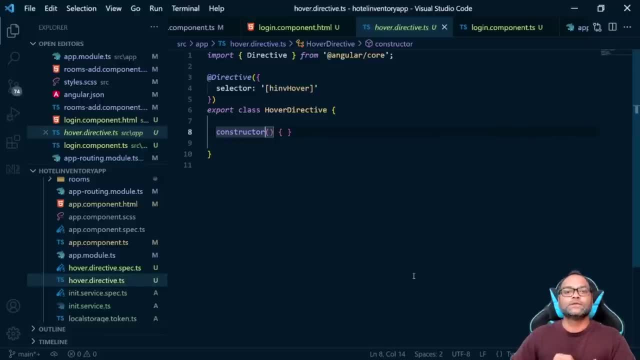 and create a folder. so or relatively we will do that later, or relatively we will do that later, or relatively we will do that later. so so so when we talked about directive, we said: when we talked about directive, we said: when we talked about directive, we said directives are. 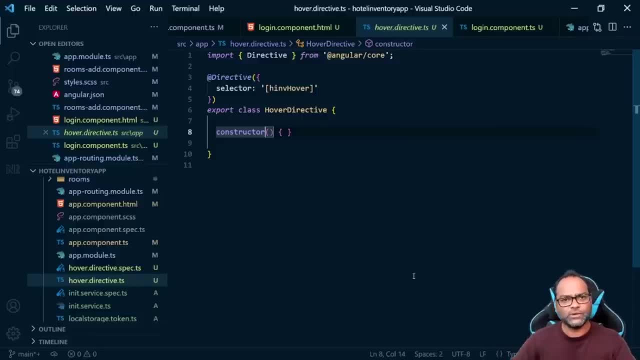 directives are directives are sorry when we talked about directive. we sorry when we talked about directive. we sorry when we talked about directive, we said directives are similar to component. said directives are similar to component. said directives are similar to component, but they will never have one thing which. 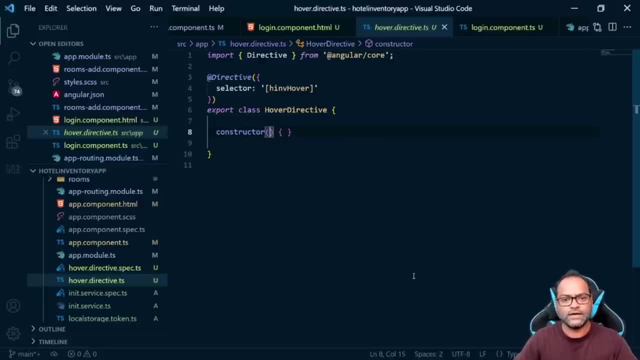 but they will never have one thing which, but they will never have one thing which is template, is template, is template. so here, uh, let's see how we can actually so. here, uh, let's see how we can actually. so here, uh, let's see how we can actually get an access to the element which is: 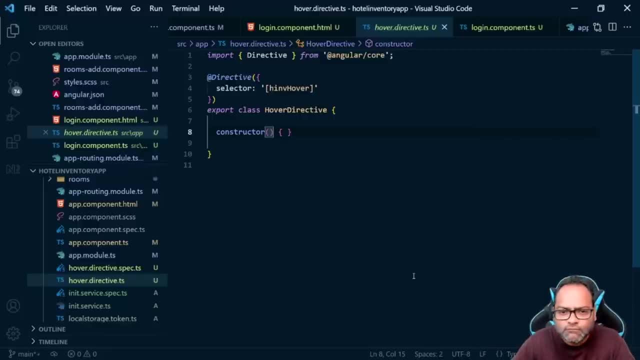 get an access to the element which is: get an access to the element which is: of course, uh, this, of course, uh, this, of course, uh, this hover directive right. so this over hover directive right. so this over hover directive right. so this over directive will be, directive will be. 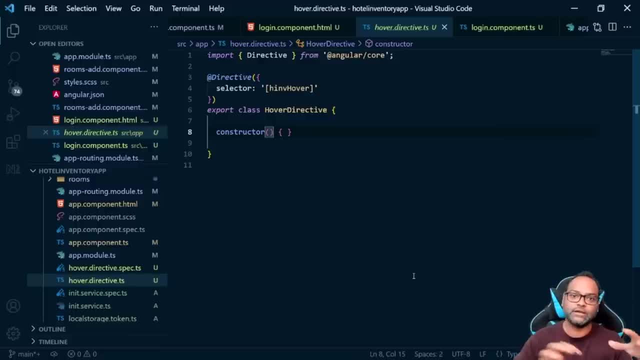 directive will be kind of a helper method to your element, kind of a helper method to your element, kind of a helper method to your element where it you can apply it. so let's see where it you can apply it. so let's see where it you can apply it. so let's see how we can do that. so 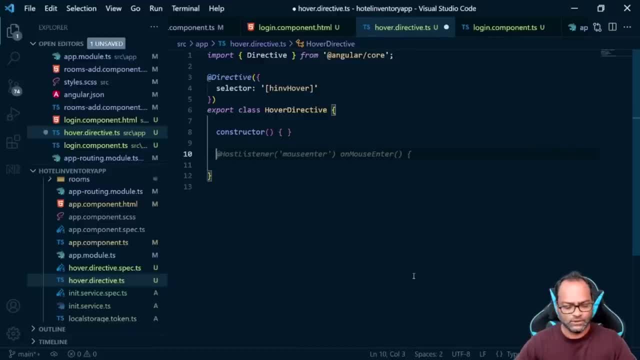 how we can do that. so how we can do that. so here uh, we will say uh, here uh, we will say uh, here uh, we will say uh, we are supposed to use host listener, but we are supposed to use host listener. but we are supposed to use host listener. but we will do that later on, but let's try. 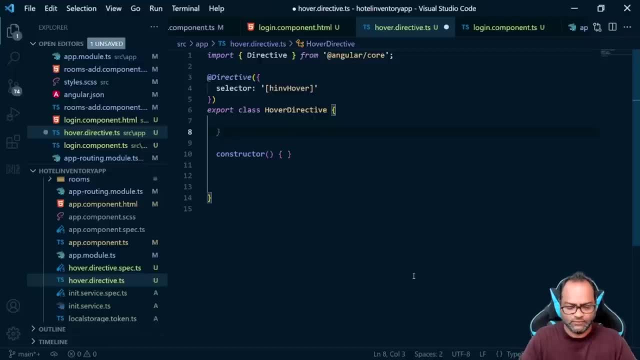 we will do that later on, but let's try. we will do that later on, but let's try to do first thing first. to do first thing first, to do first thing first. we will say: let's apply some color, let's apply some color, let's apply some color. so i'm saying the 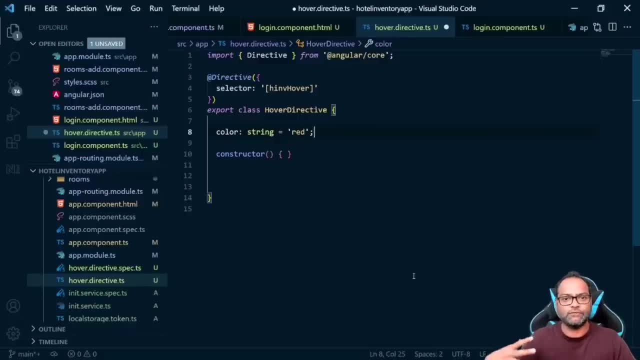 so i'm saying the, so i'm saying the by default, your by default, your by default, your, when, whenever we try to when, whenever we try to when, whenever we try to, let's say when we apply this particular, let's say when we apply this particular, let's say when we apply this particular directory. we are not talking about right. 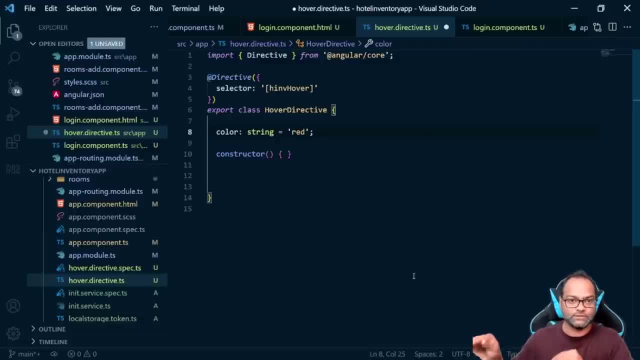 directory. we are not talking about right directory. we are not talking about, right now, how to use host listener. i mean host now. how to use host listener. i mean host now. how to use host listener. i mean host listener. there's something which we'll listener. there's something which we'll 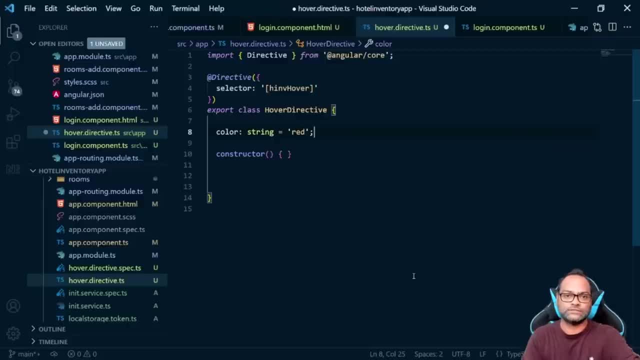 listener. there's something which we'll talk about, so let's not get confused. so talk about. so let's not get confused, so talk about. so let's not get confused. so, right now, we are just trying to see. right now, we are just trying to see, right now we are just trying to see once we apply this particular directive. 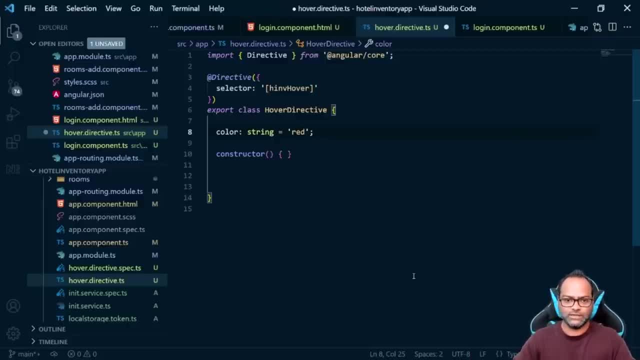 once we apply this particular directive. once we apply this particular directive, it should change the background color to it, should change the background color to it, should change the background color to red, red, red, right. so right, so right. so here, what we can do is we can implement. 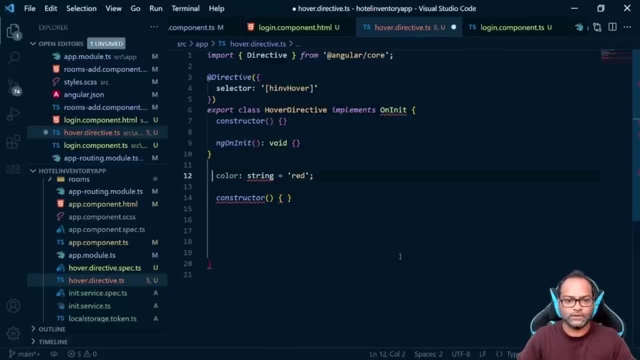 here. what we can do is we can implement here. what we can do is we can implement uh, implement uh on init lifecycle. look the reason we can actually use lives. uh, the reason we can actually use lives, uh, the reason we can actually use lives, uh ng on it or all the lifecycle looks is 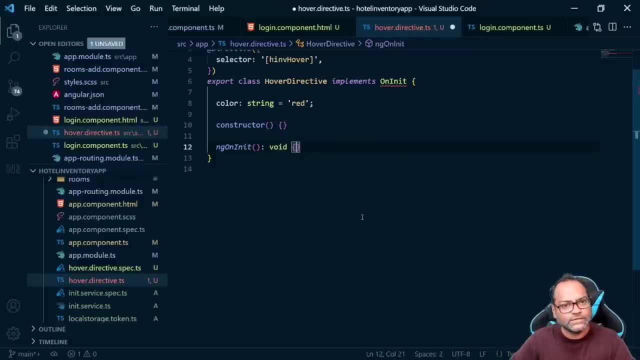 ng on it or all the lifecycle looks is ng on it or all the lifecycle looks is, as we said, directives is similar to what. as we said, directives is similar to what. as we said, directives is similar to what your components are apart from this. your components are apart from this. 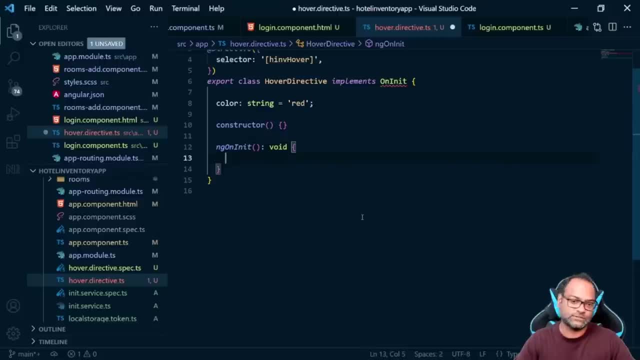 your components are apart from this template, but it can still go ahead and template, but it can still go ahead and template, but it can still go ahead and use all the lifecycle looks as well. so use all the lifecycle looks as well. so use all the lifecycle looks as well. so here, uh. now what we need is we need uh. 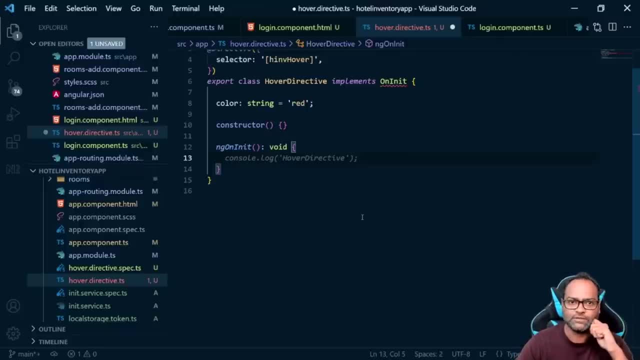 here, uh now. what we need is: we need uh here, uh. now. what we need is: we need uh, this color to be applied to the element, this color to be applied to the element, this color to be applied to the element which is available outside right, which is available outside right. 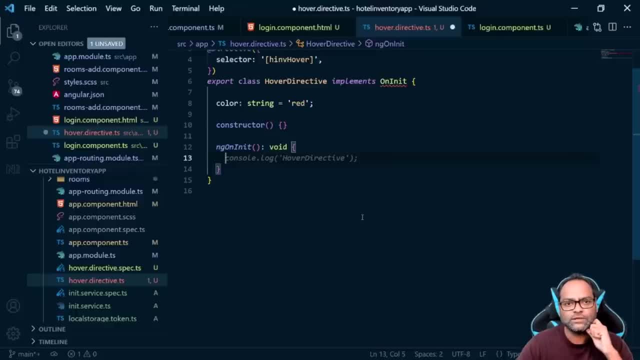 which is available outside right. it's uh, it's uh, it's uh. i mean how we can do that, i mean how we can do that, i mean how we can do that. so let's see, so, let's see, so, let's see. so here, uh, we will see, we will provide. 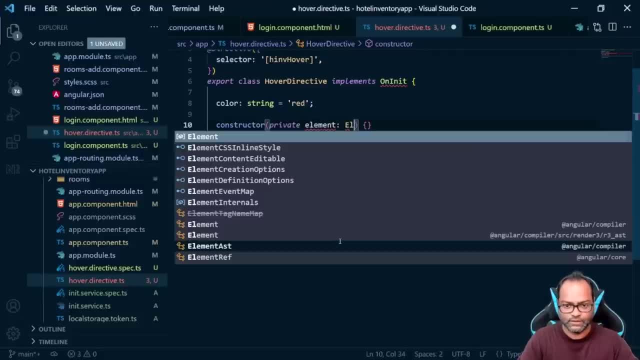 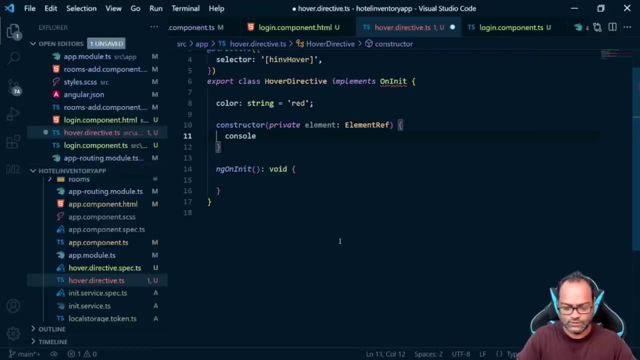 we will inject, we will inject, we will inject. element with this type of element- ref. element with this type of element- ref. element with this type of element- ref. and. and, and, let's, let's, let's do a consolelog here, do a consolelog here, do a consolelog here and see what this element is. 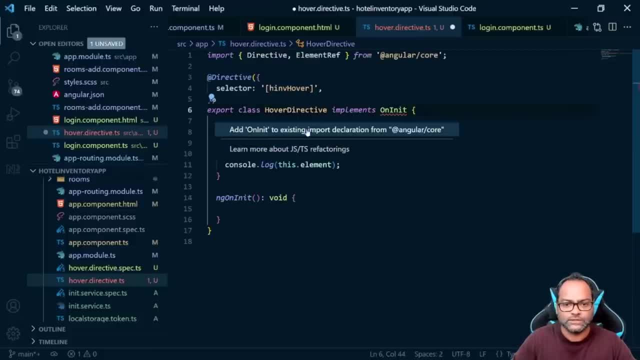 on in it, on in it, on in it. why okay? so let me just add this. so what? why okay? so let me just add this. so what? why okay? so let me just add this: so what we have done so far? we have just. we have done so far, we have just. 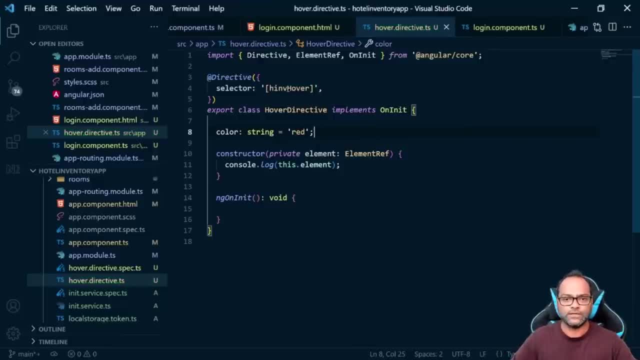 we have done so far. we have just injected element ref and we have just injected element ref and we have just injected element ref and we have just done consolelog. now let's square and done consolelog. now let's square and done consolelog. now let's square and apply this particular directive. how to 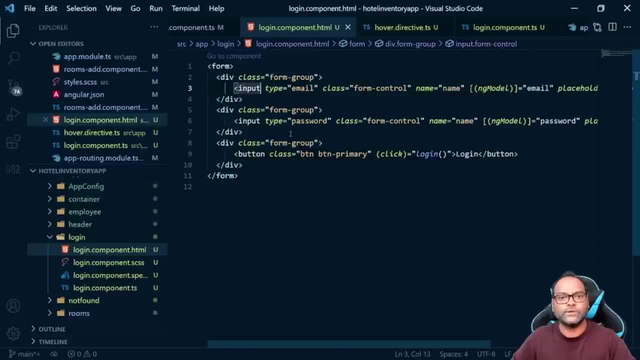 apply this particular directive. how to apply this particular directive. how to apply it so we can go to the component. apply it so we can go to the component. apply it so we can go to the component. this input element is where i want to. this input element is where i want to. 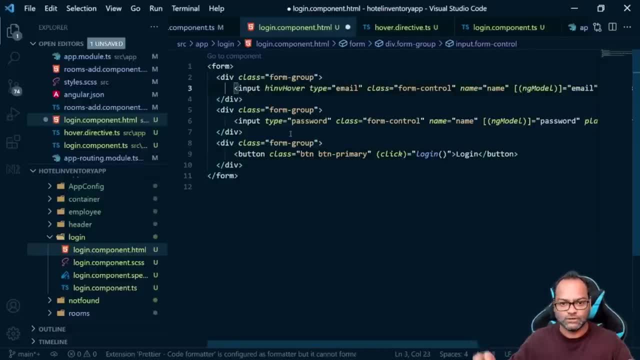 this input element is where i want to apply it. apply it. apply it. just add it like this: h i and v over. just add it like this: h i and v over. just add it like this: h i and v over, and let's apply it here as well. so we 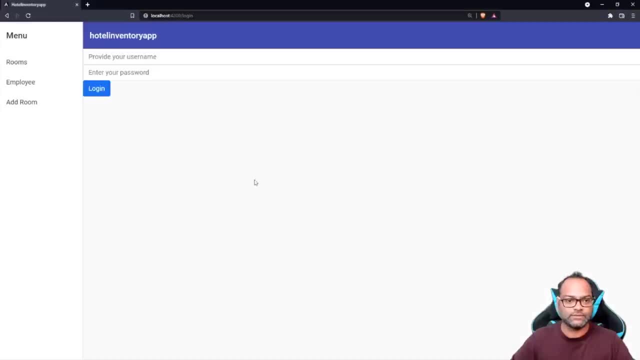 and let's apply it here as well. so we, and let's apply it here as well. so we are we, we can use directives. it's a are we? we can use directives. it's a are we? we can use directives. it's a reusable thing. so let's inspect. 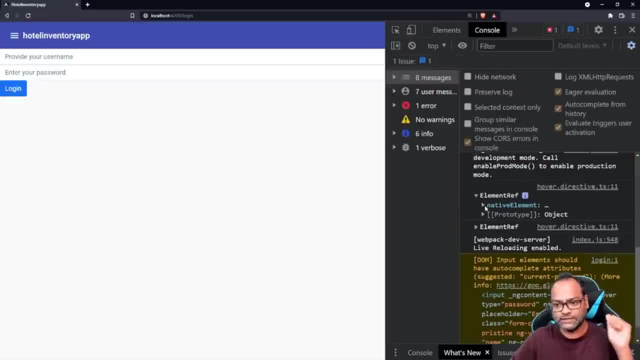 reusable thing, so let's inspect. reusable thing, so let's inspect. let's go to console, and here is the. let's go to console, and here is the. let's go to console. and here is the interesting thing which we want to, interesting thing which we want to. 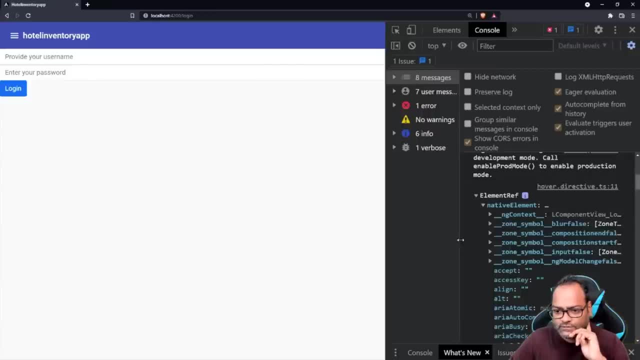 interesting thing which we want to discuss about, so you can see, discuss about, so you can see, discuss about, so you can see uh native element. it gives gives you uh native element. it gives gives you uh native element. it gives gives you access to the native element. so what? 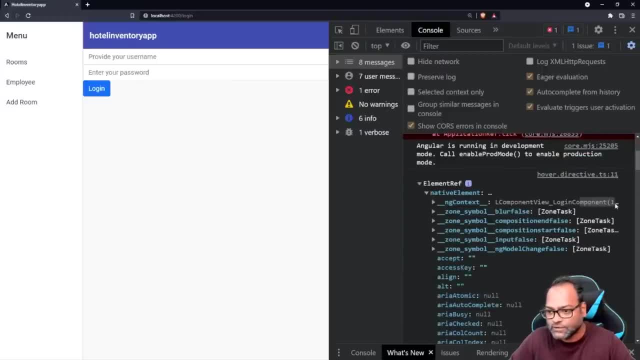 access to the native element. so what access to the native element? so what? to simplify this? i mean, of course we can to simplify this. i mean, of course we can to simplify this. i mean, of course we can see that. okay, it is referring to the. see that. okay, it is referring to the. 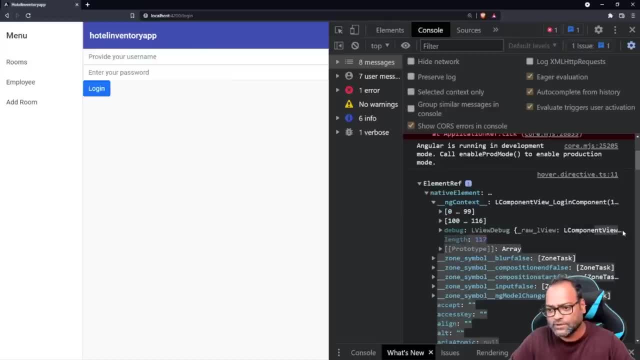 see that, okay, it is referring to the login component. you can see the context login component. you can see the context login component. you can see the context. so it says, okay, it is coming from. so it says, okay, it is coming from. so it says, okay, it is coming from something called login component. so to 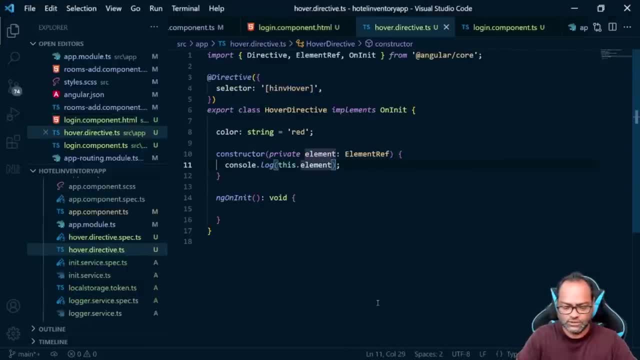 something called login component, so to something called login component. so to simplify it, simplify it. simplify it. let's go ahead and say this element dot. let's go ahead and say this element dot. let's go ahead and say this element dot, native element, native element, native element, and let's see what we get. 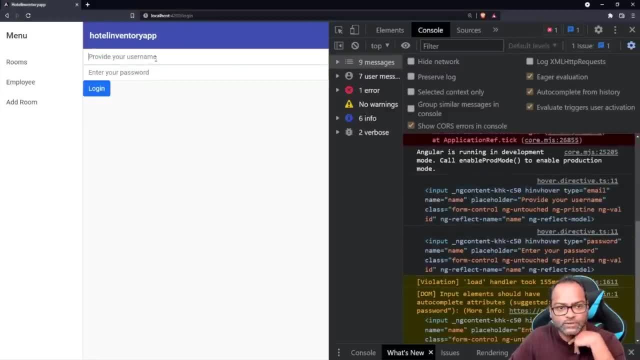 and let's see what we get. and let's see what we get. so here you can see you are actually so here you can see you are actually. so here you can see you are actually getting this input element, how you can getting this input element, how you can. 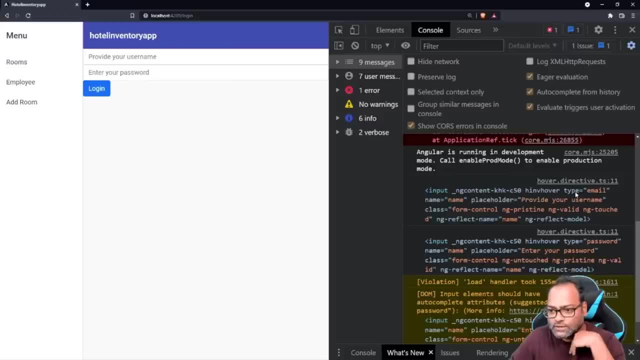 getting this input element, how you can actually just go ahead and actually just go ahead and actually just go ahead and see, i mean you can just click on it. see, i mean you can just click on it. see, i mean you can just click on it and see: okay, this is the email and this. 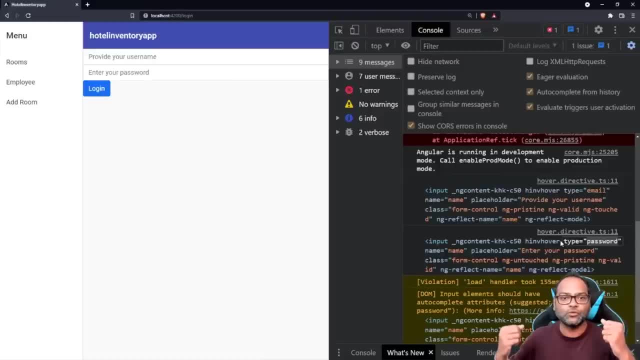 and see: okay, this is the email and this is the password, so we are actually is the password, so we are actually is the password. so we are actually getting the reference to the element, on getting the reference to the element, on getting the reference to the element on which you are applying the directive. so which you are applying the directive, so which you are applying the directive, so this element ref will give the access to this element. ref will give the access to this element ref will give the access to the element. now you can actually go ahead. the element: now you can actually go ahead. 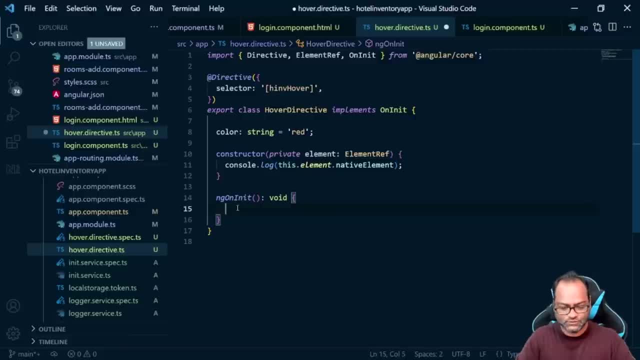 the element. now you can actually go ahead and do whatever you want to with this, and do whatever you want to with this and do whatever you want to with this particular element. let's do this, so i can. particular element. let's do this, so i can particular element. let's do this so i can say this: dot element, dot- native element. 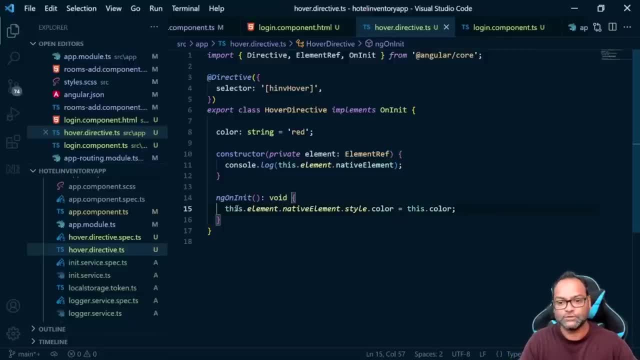 say this dot element, dot native element, say this dot element, dot native element. and i can just variance the two dot style and i can just variance the two dot style and i can just variance the two dot style. dot color is equal to this dot color, dot color is equal to this dot color. 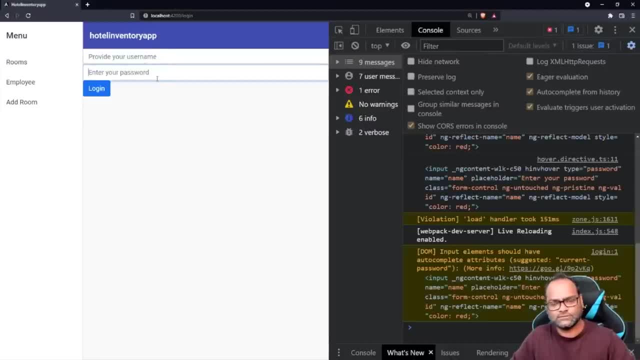 dot color is equal to this dot color. let's see, let's see, let's see. but okay, nothing happened because of, but okay, nothing happened because of, but okay, nothing happened because, of course, color is not a property, so i can. course, color is not a property, so i can. 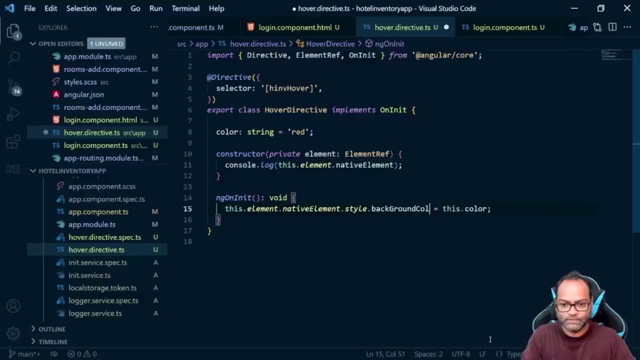 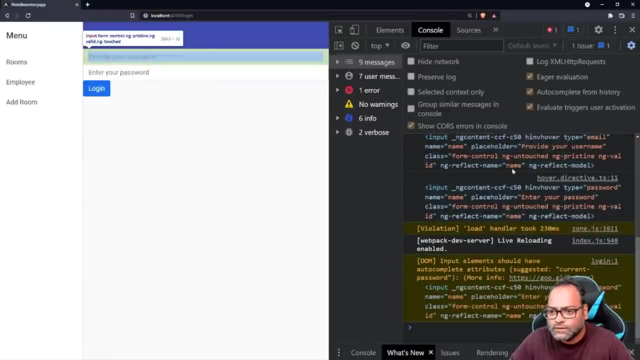 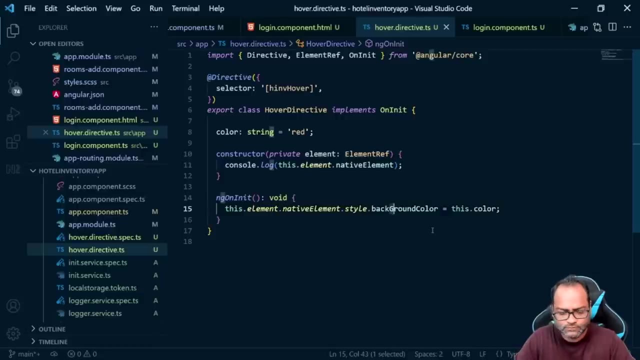 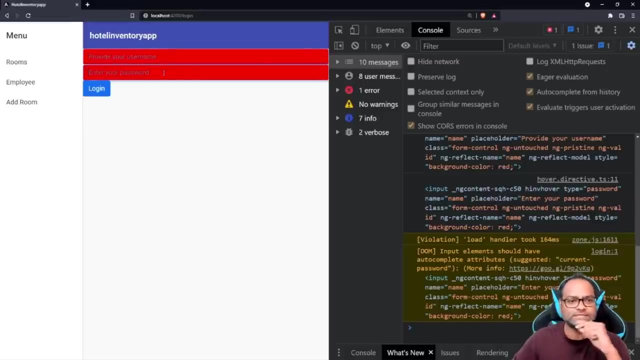 course color is not a property, so i can say back ground, say back ground, say back ground color. let's see. okay, so it was small g, so now you can see i. okay, so it was small g, so now you can see i. okay, so it was small g, so now you can see i. i just changed the background color of 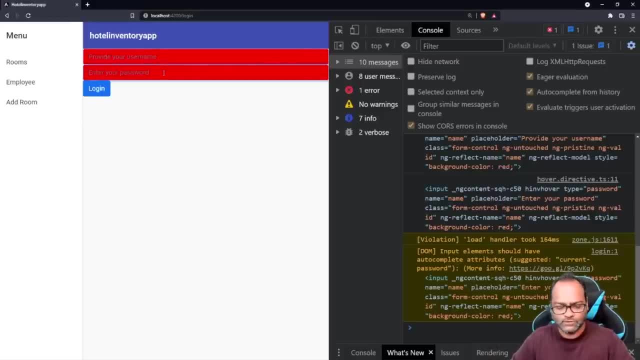 i just changed the background color of, i just changed the background color of this particular, this particular, this particular input control by using the style input control, by using the style input control, by using the style property directly, but you can, of course, property directly, but you can, of course. 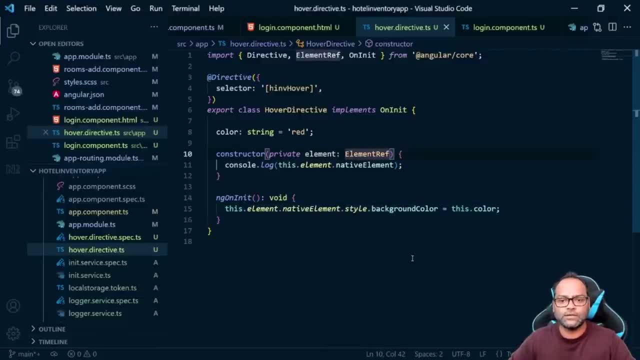 property directly. but you can, of course, do better. you can actually go ahead and do better. you can actually go ahead and do better. you can actually go ahead and do it using. do it using. do it using: the document object right, so you can go, the document object right, so you can go. 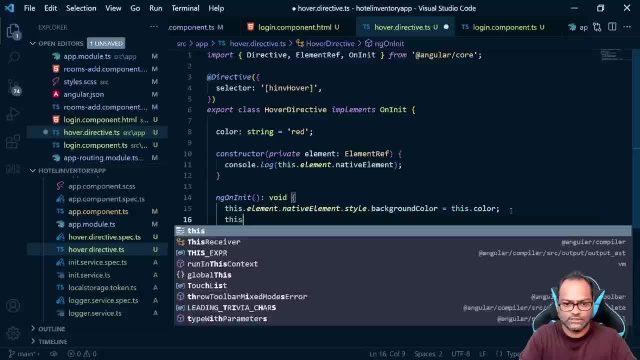 the document object right, so you can go ahead and do ahead and do ahead and do uh using that. so let me show you an uh using that. so let me show you an uh using that. so let me show you an example so i can say example, so i can say: 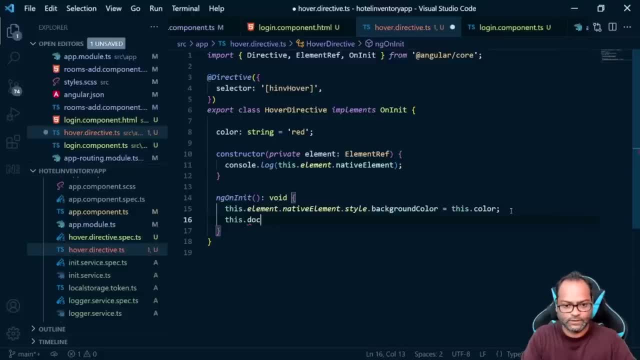 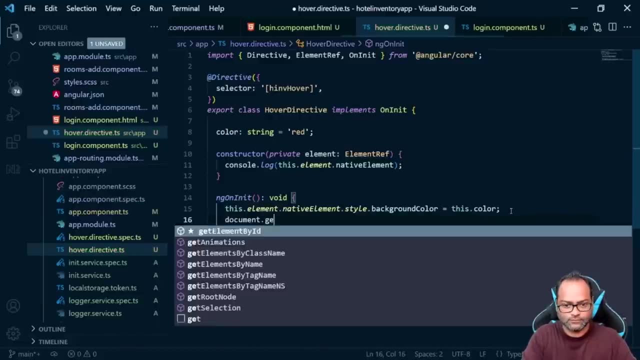 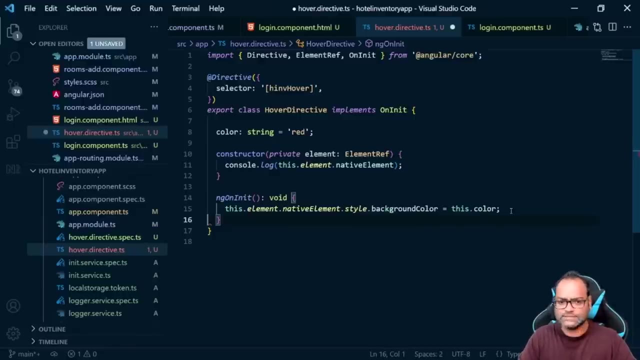 example, so i can say this dot document, or let me, or let me, or let me use the use, the use the class actually. uh, there is a class, which class actually. uh, there is a class which class actually. uh, there is a class which is available, so is available, so. 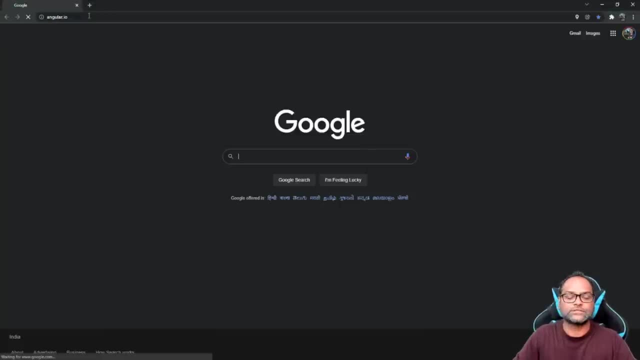 is available. so, uh, let's, uh, let's, uh, let's grab that class. i can just go to angular, grab that class. i can just go to angular, grab that class. i can just go to angular. dot io, uh, it's document. dot io, uh, it's document. 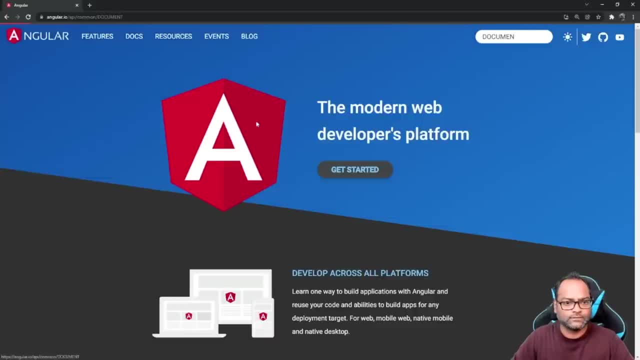 dot io. uh, it's document. i'm not wrong. yeah, i'm not wrong. yeah, i'm not wrong. yeah, okay, so, anyways, that's, that's the api. okay, so, anyways, that's, that's the api. okay, so, anyways, that's, that's the api which i wanted, so you can actually just 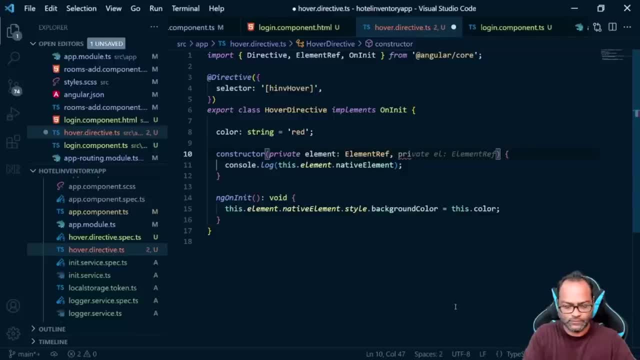 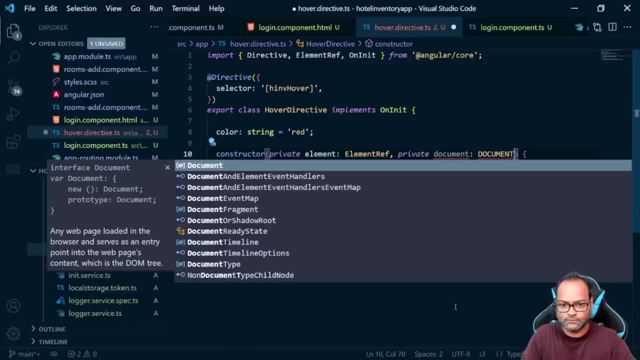 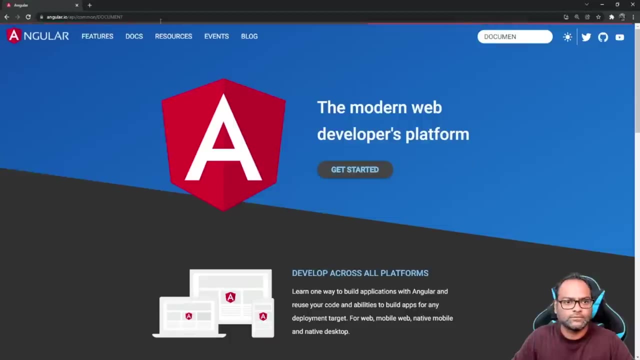 which i wanted, so you can actually just which i wanted, so you can actually just inject this private document, which will be type of document, document which will be type of document. let's see, let's see, let's see it's an, it's an, it's an injection. okay. 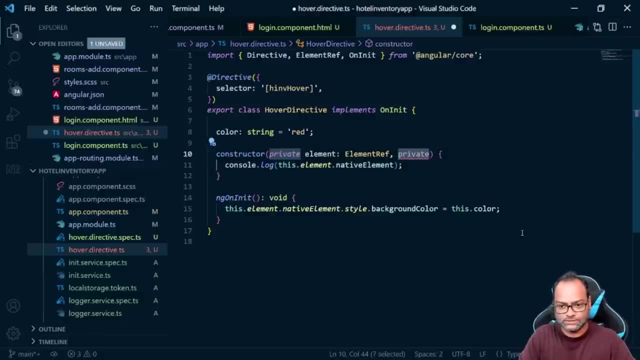 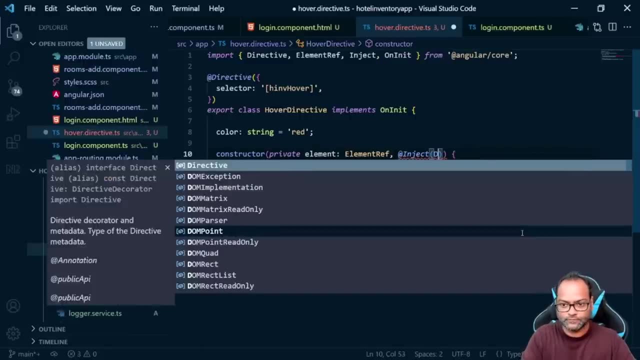 injection, okay, injection. okay, it's an injection token, so i can uh do it's an injection token, so i can uh do it's an injection token, so i can uh do something like this: add the rate. something like this: add the rate, something like this, add the rate inject. 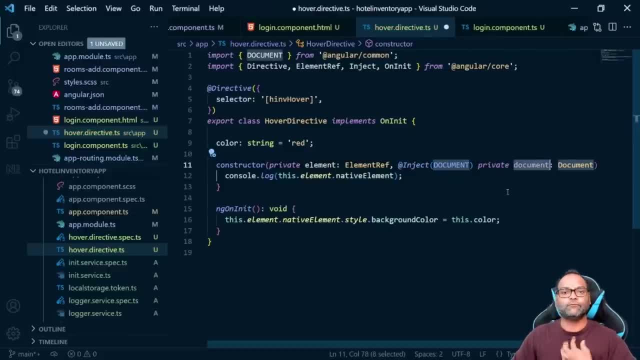 now, now, using this document. so, uh, using this document. so, uh, using this document. so, uh, let's talk about this document object. let's talk about this document object. let's talk about this document object which we are talking about, so which we are talking about, so which we are talking about, so, remember, in web. so let's say, if i inspect, 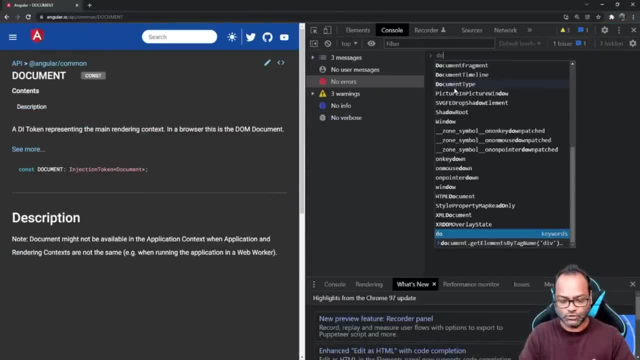 remember in web. so let's say: if i inspect, remember in web. so let's say: if i inspect, this i mean this is normal html. this i mean this is normal html. this, i mean this is normal html. if i try to access this document, right, if i try to access this document right. 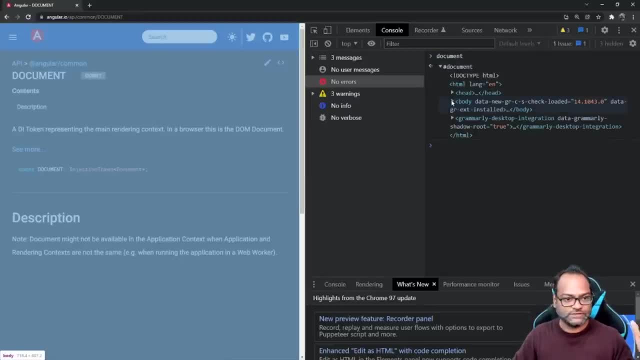 if i try to access this document, right, so it gives me access to the entire. so it gives me access to the entire. so it gives me access to the entire page. i mean whatever control which is page. i mean whatever control which is page. i mean whatever control which is available here so you can see, i get. 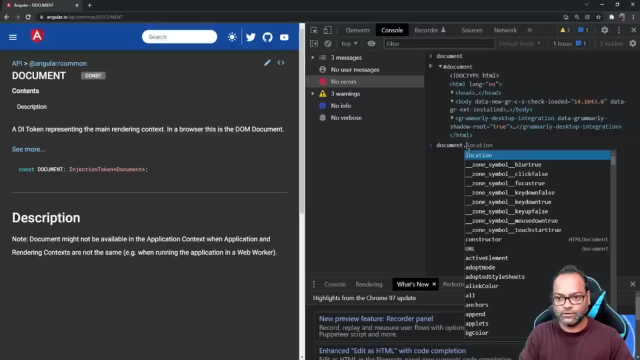 available here so you can see. i get available here so you can see i get access to html head body everything and access to html head body everything. and access to html head body everything. and by using document dot, get element by id. by using document dot, get element by id. 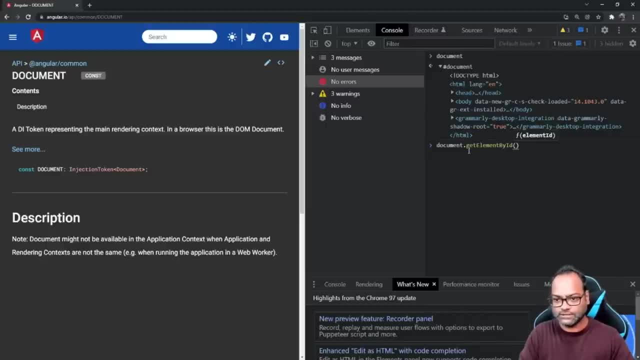 by using document dot. get element by id. these are some apis which are which is: these are some apis which are which is. these are some apis which are which is available here, so i can just word. and available here, so i can just word. and available here, so i can just word and say i can get access to any element. 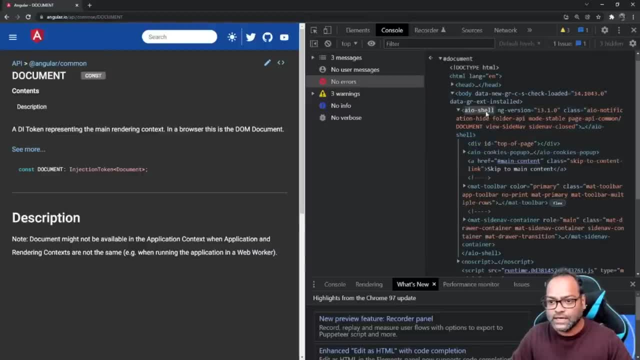 say i can get access to any element, say i can get access to any element which is available here, for example, which is available here, for example, which is available here, for example. let's say this aio shell, right, so this. let's say this aio shell, right, so this. 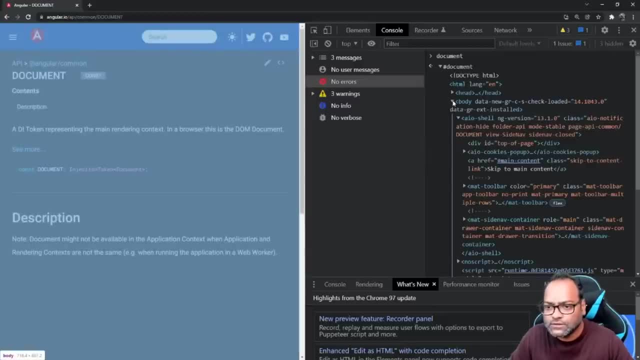 let's say this: aio shell, right. so this is one of the element. if i do this, okay, is one of the element. if i do this, okay is one of the element. if i do this, okay, uh, this is not id. oh, okay, sorry, this is uh, this is not id. oh, okay, sorry, this is. 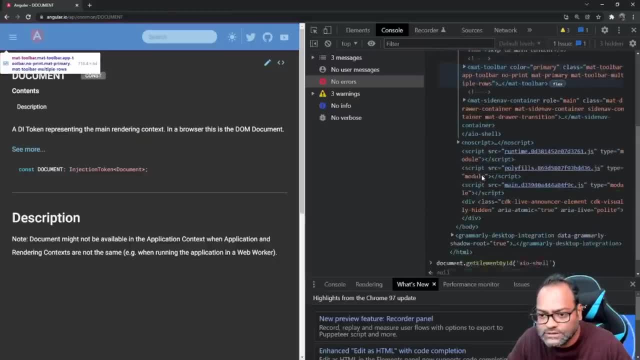 uh, this is not id. oh okay, sorry, this is an uh an uh an uh tag. this is not an id. let's search for tag. this is not an id. let's search for tag. this is not an id. let's search for something which is an id. 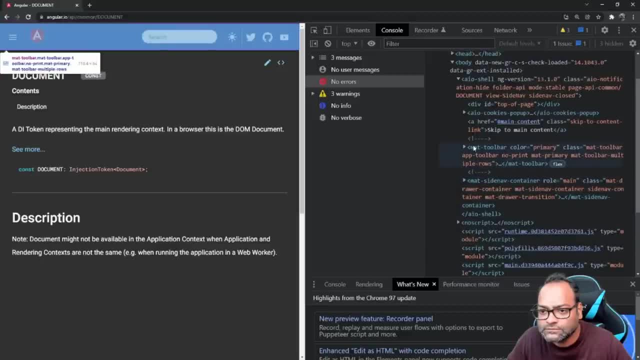 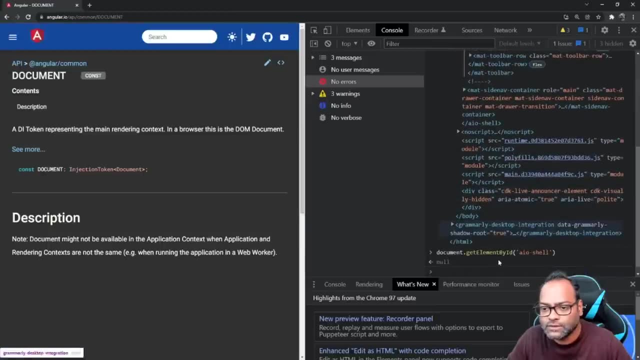 something which is an id and class this. okay, there is nothing, there's no id. so there's no id, so there's no id. so let's try to do this mac toolbar. let's try to do this mac toolbar. let's try to do this mac toolbar by using: 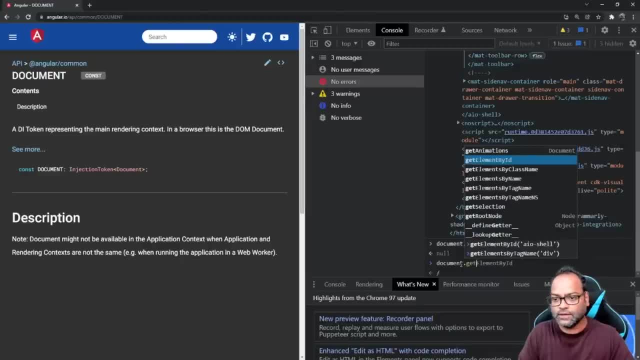 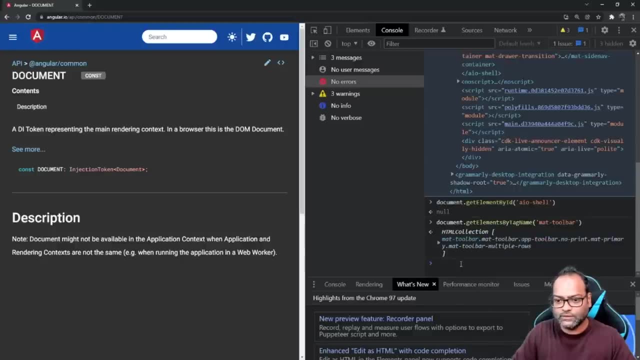 by using: by using: not document, not document, not document, dot, get, dot, get, dot. get. element by tag, element by tag, element by tag name, name, name, and i can just put the tag name here, and and i can just put the tag name here, and and i can just put the tag name here and you can see i can get the access to the. 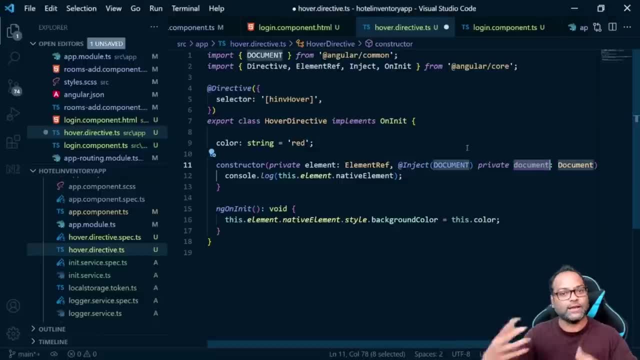 you can see, i can get the access to the. you can see, i can get the access to the html element. so this is a web api. so this html element, so this is a web api. so this html element. so this is a web api. so this document is actually a wrapper around. 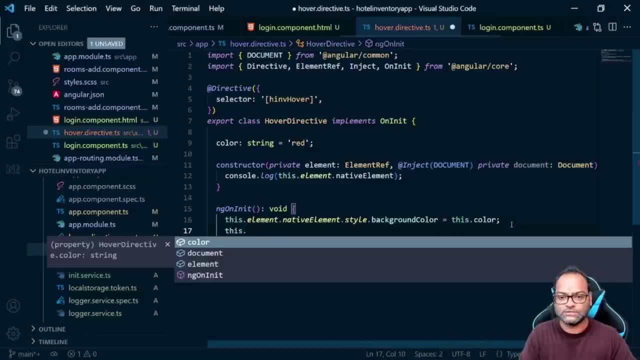 document is actually a wrapper around. document is actually a wrapper around the same. and by using this, we can the same, and by using this, we can the same. and by using this, we can actually just simplify this. so you can actually just simplify this, so you can actually just simplify this, so you can say this: dot, document, dot. 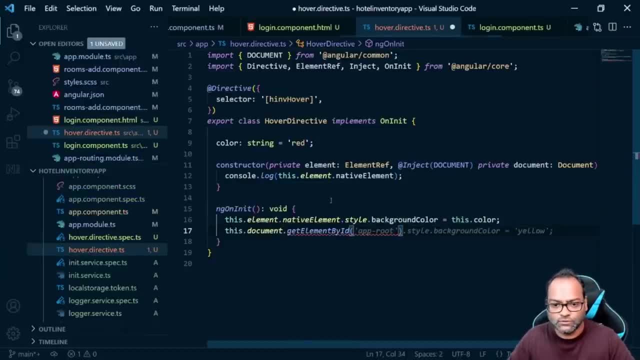 say this dot document, dot. say this dot document dot. uh, uh, uh. inside get element by id. so not getting inside get element by id. so not getting inside get element by id, so not getting get element by id. but i can just do get element by id, but i can just do. 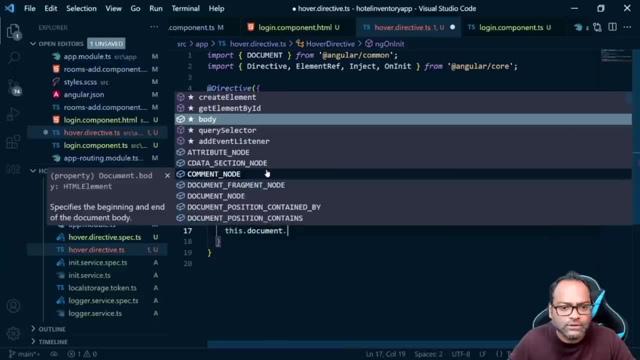 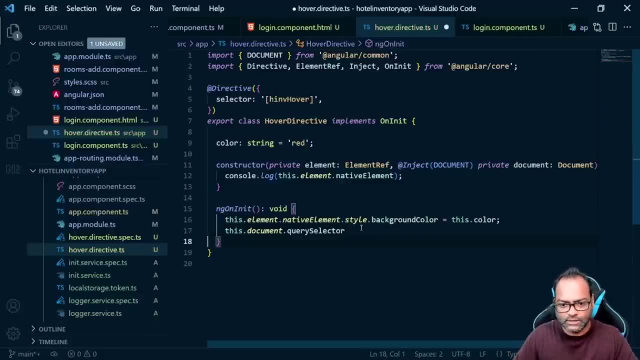 get element by id. but i can just do. let's see what we can use here. create element. create element. create element very selected. let's see if i can pass very selected. let's see if i can pass very selected. let's see if i can pass uh element here. 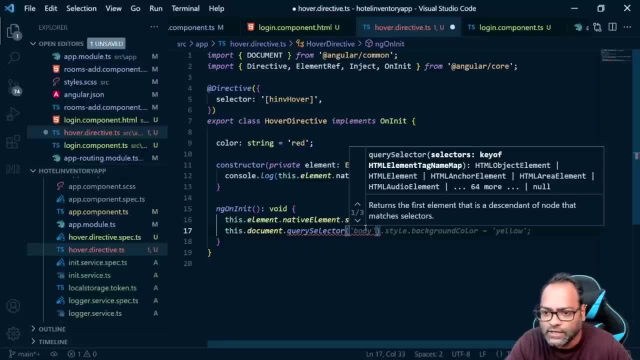 uh, element here. uh, element here. let's see what it takes, so it stays. uh, let's see what it takes, so it stays. uh, let's see what it takes, so it stays. uh, html of type or html element as well. so html of type or html element as well. so. 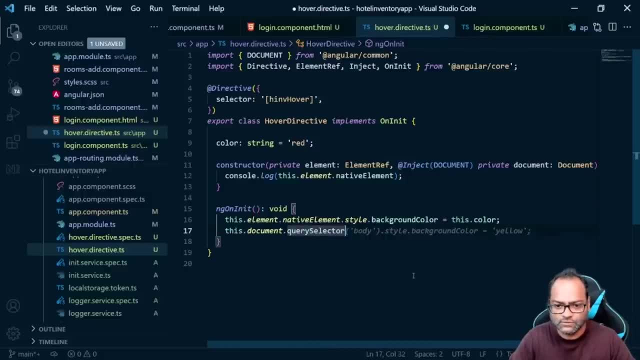 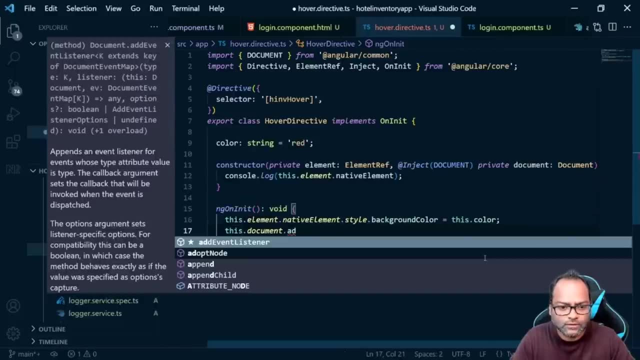 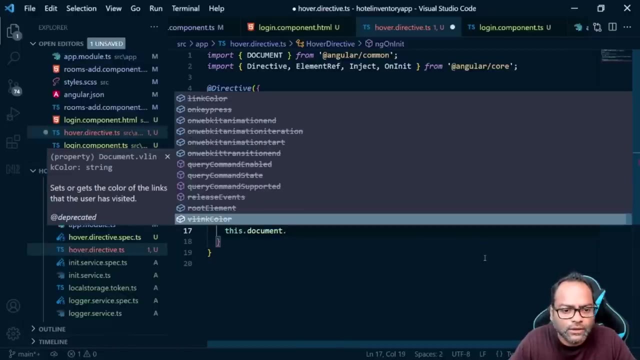 html of type or html element as well. so let's see, let's see, let's see. probably this is not the one. also, we are probably this is not the one. also, we are probably this is not the one also we are looking for. okay, there are a few more properties. i'm 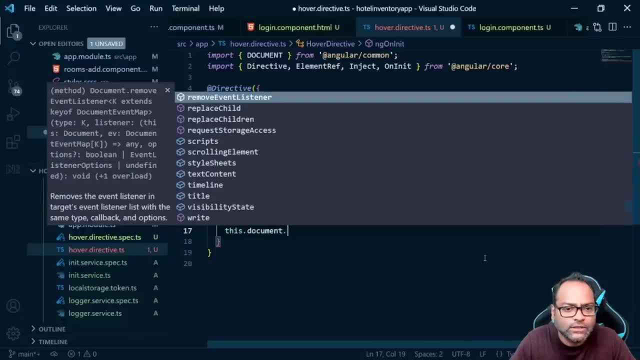 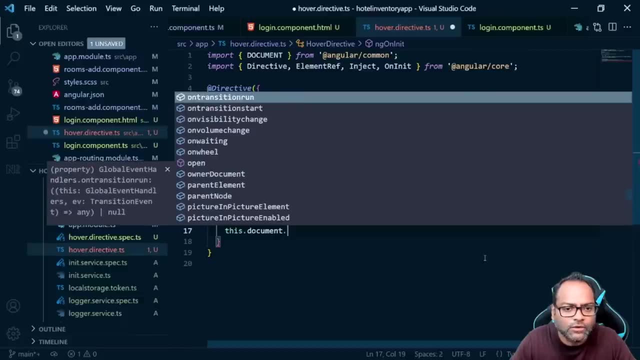 okay, there are a few more properties. i'm okay, there are a few more properties, i'm looking for one. let's see looking for one. let's see looking for one. let's see stylesheet replace: very selective different plugins: okay, very selective different plugins. okay, very selective different plugins- okay. on. 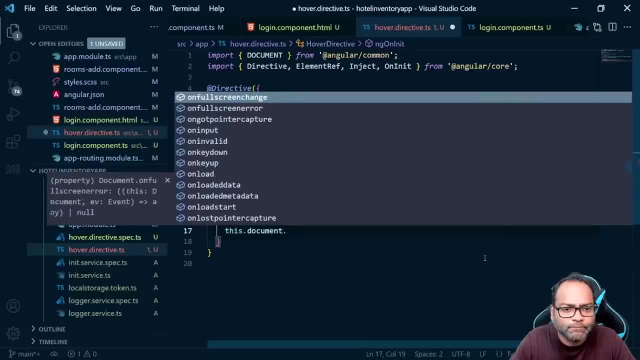 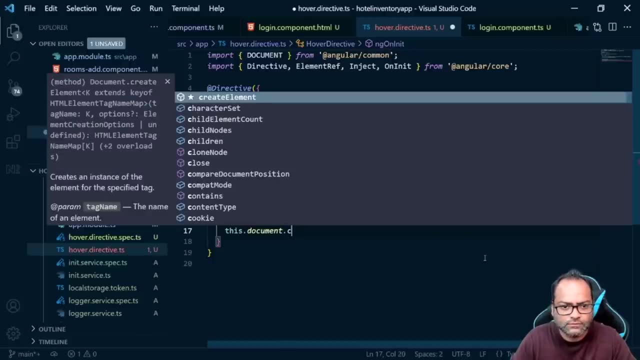 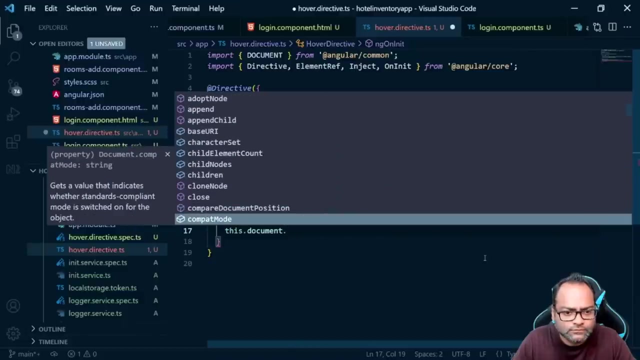 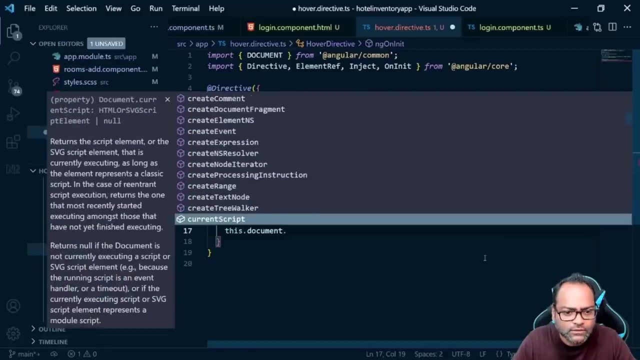 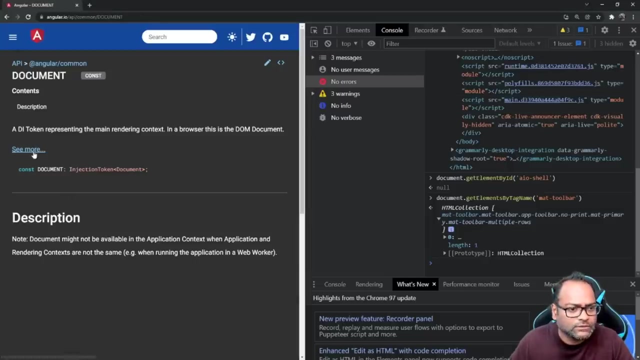 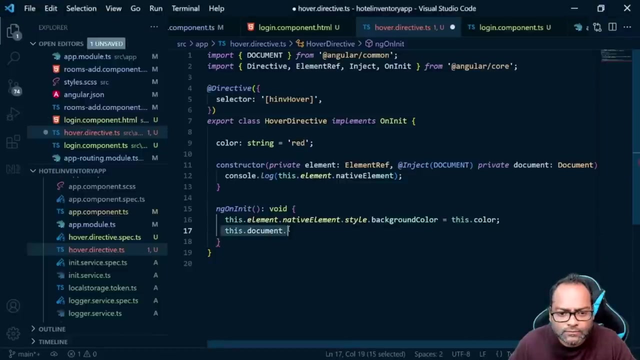 okay on. okay on something related to class. getting that. something related to class. getting that, something related to class. getting that. you are saying: when child contains cookies, when child contains cookies, when child contains cookies create, when child contains cookies, create element. okay, let's see document. so, uh, let's go ahead and see this. i mean 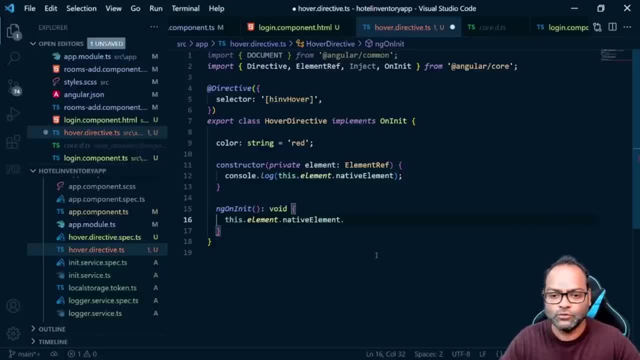 so, uh, let's go ahead and see this. i mean so, uh, let's go ahead and see this. i mean using multiple ways. so there are using multiple ways, so there are using multiple ways. so there are something which we can do set, something which we can do set. something which we can do, set uh. we can also see that we can also uh. we can also see that. we can also see that we can also see that we can uh. we can also see that we can also see that we can actually do it using the dom. 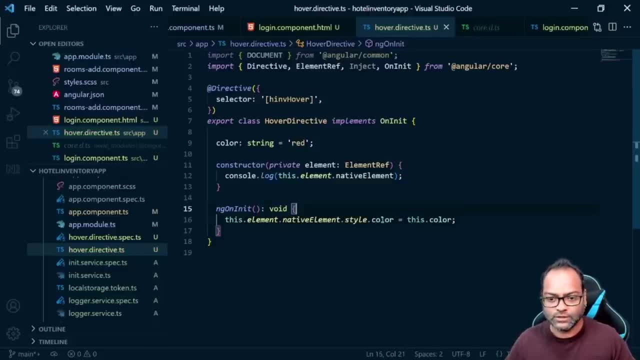 actually do it using the dom, actually do it using the dom, or we can actually i mean the this way, or we can actually i mean the this way, or we can actually i mean the this way. stylecolor or background color which we. stylecolor or background color which we. 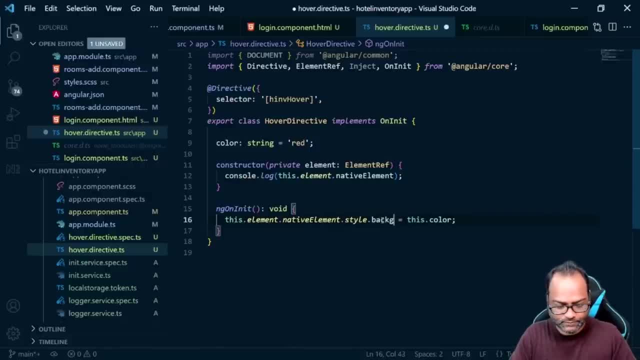 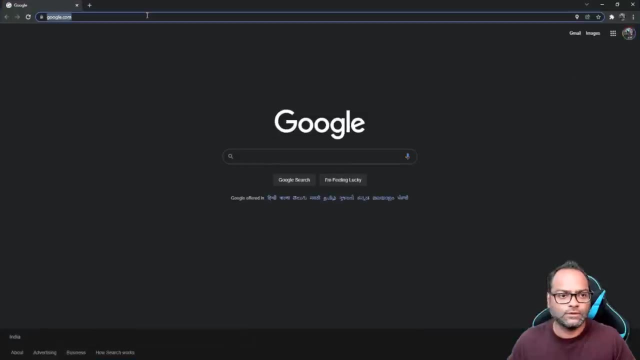 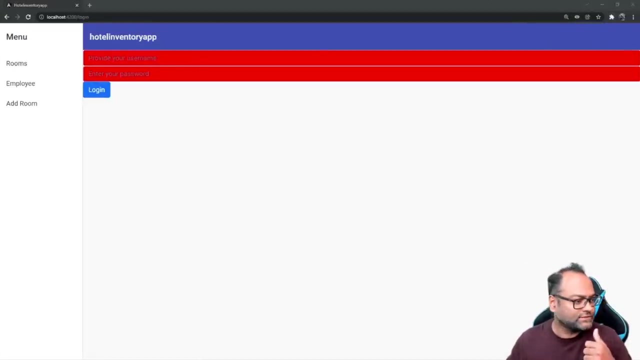 stylecolor or background color, which we have seen, have seen, have seen so back background color, and let's see the application again now. let's see the application again now. let's see the application again now. yeah, yeah, yeah, but there is another way as well, another, but there is another way as well, another. 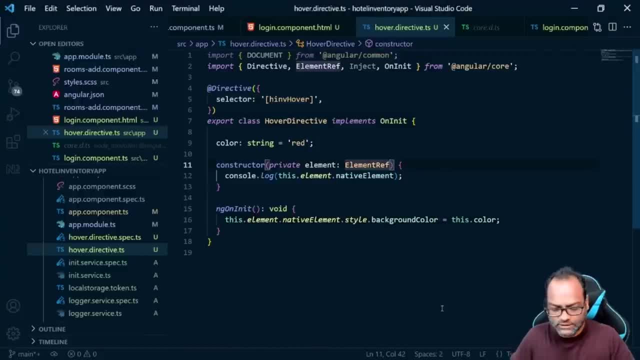 but there is another way as well, another way possible. let's see that. so there is way possible. let's see that. so there is way possible. let's see that. so there is another api which is available, and we another api which is available, and we another api which is available, and we can also use that api to simplify this. 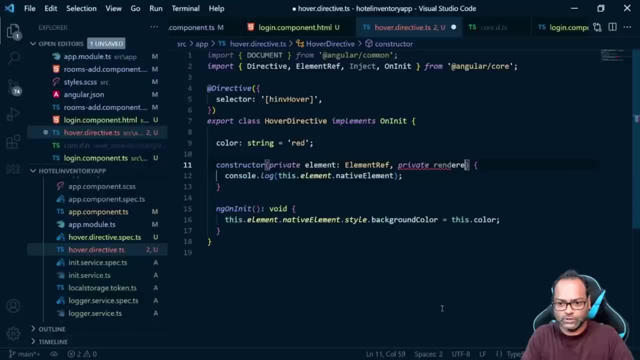 can also use that api to simplify this. can also use that api to simplify this. which is known as a renderer 2, so i can. which is known as a renderer 2, so i can. which is known as a renderer 2, so i can just do renderer. 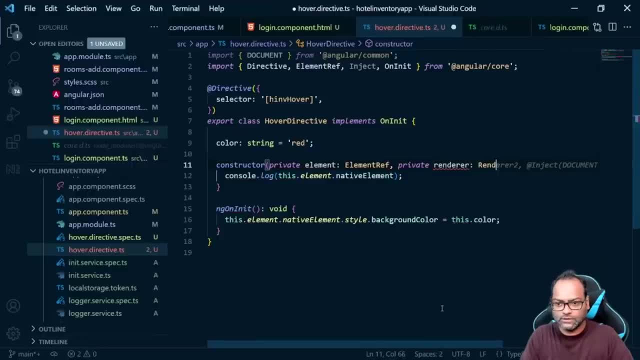 or just name it: renderer and you'll see. or just name it renderer and you'll see. or just name it renderer and you'll see: renderer 2. why renderer 2? because renderer 2 is. why renderer 2? because renderer 2 is because there is already a api called. 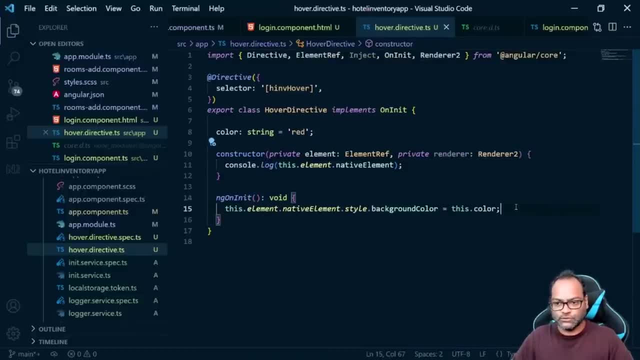 because there is already a api called. because there is already a api called renderer, so renderer, so renderer, so renderer 2 is something which you can use. renderer 2 is something which you can use. renderer 2 is something which you can use and we can actually simplify this by: 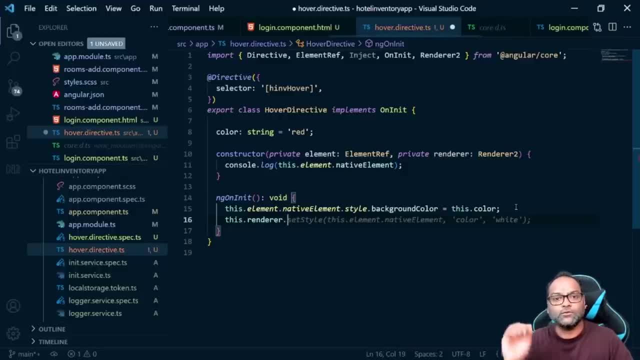 and we can actually simplify this by- and we can actually simplify this by using renderer api. so you can say using renderer api. so you can say using renderer api. so you can say renderer dot, and now you get met access. renderer dot, and now you get met access. 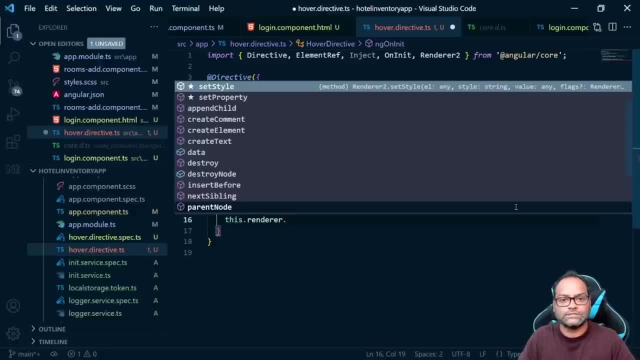 renderer dot and now you get met access to all the methods there are set style to all the methods there are set style to all the methods. there are set style set property. so this is uh something set property. so this is uh something set property. so this is uh something which is. 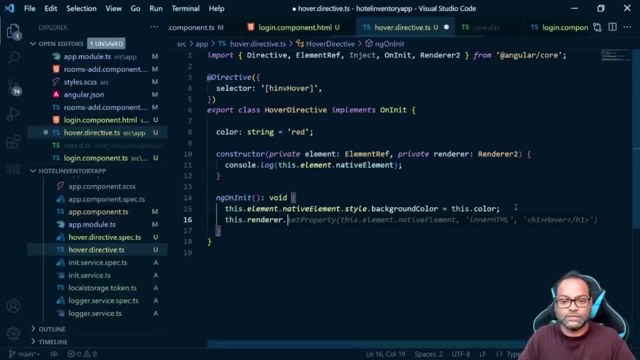 which is, which is property, if i'm not wrong yet, property if i'm not wrong yet property, if i'm not wrong yet. oh sorry, this is the style. oh sorry, this is the style, oh sorry, this is the style. so you can say set style and the first. 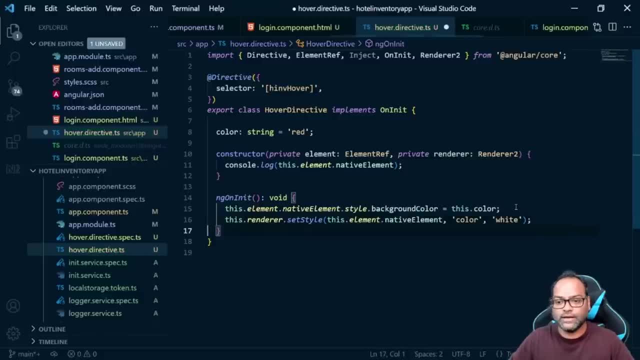 so you can say set style, and the first, so you can say set style, and the first parameter which we have to pass is the parameter which we have to pass is the parameter which we have to pass is the element, so we can pass the element, and element, so we can pass the element. and. 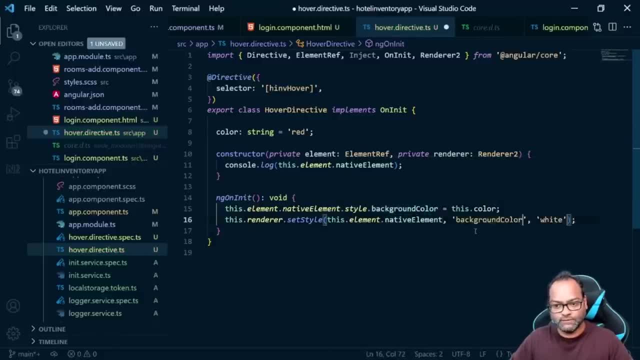 element, so we can pass the element and then the, then the, then the second parameter would be the property. second parameter would be the property. second parameter would be the property which you want to change and the third which you want to change, and the third which you want to change, and the third parameter will be the actual value. so i 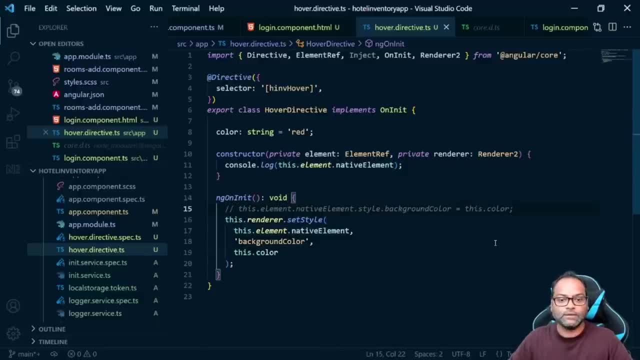 parameter will be the actual value. so i parameter will be the actual value, so i can save with this, can save with this, can save with this dot color, dot color, dot color, and let's see, and let's see, and let's see, we will achieve the same thing. so we. 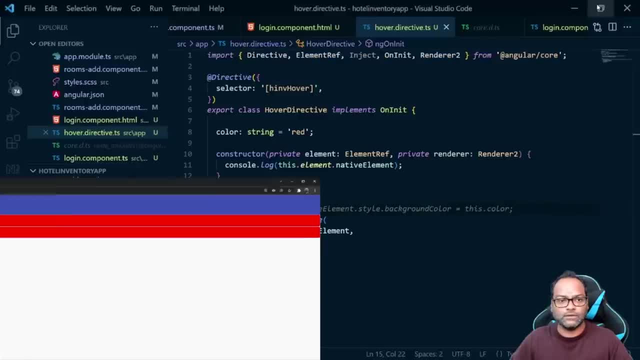 we will achieve the same thing. so we, we will achieve the same thing. so we have now, have now, have now, same available, same available, same available. uh, the background color available as uh, the background color available as uh. the background color available as red, red, red. so this is, this is the same uh, simple. so this is, this is the same, uh simple. so this is this is the same, uh simple. ap a simple example, right. how you can ap a simple example, right. how you can ap a simple example, right, how you can actually be change the behavior of your, actually be change the behavior of your. 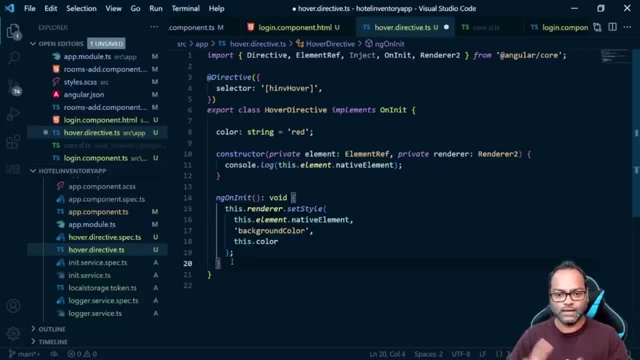 actually be. change the behavior of your dom element by using dom element, by using dom element, by using the element ref and the renderer, the element ref and the renderer, the element ref and the renderer. what in case we want to actually do? what in case we want to actually do? 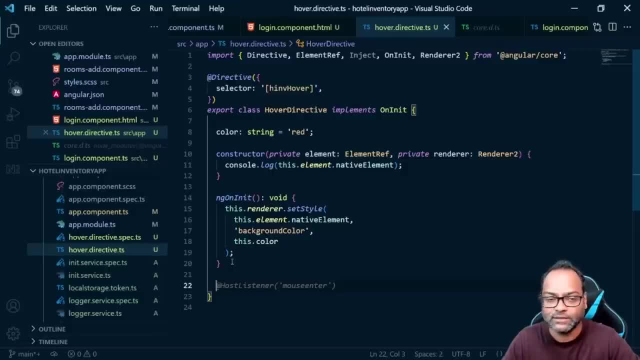 what, in case, we want to actually do something based on the event, which will something based on the event, which will? something based on the event which will happen on your parent control, happen on your parent control, happen on your parent control. a simple example can be, let's say, uh. 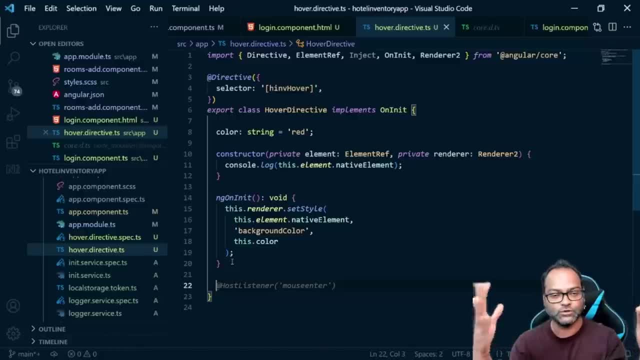 a simple example can be. let's say: uh. a simple example can be: let's say: uh, whenever you hover above your rows, whenever you hover above your rows, whenever you hover above your rows, right so you have a table. and whenever, right so you have a table. and whenever 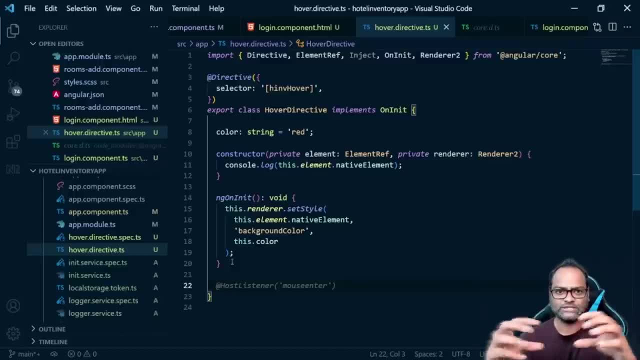 right. so you have a table and whenever you hover above your rows, you should you hover above your rows, you should you hover above your rows, you should probably change or highlight that, probably change or highlight that, probably change or highlight that particular row. so common example, right. particular row, so common example, right. 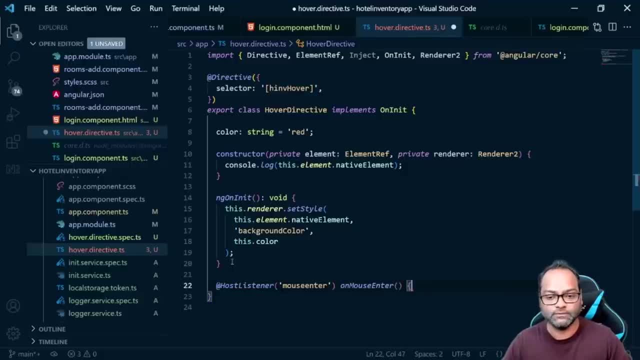 particular row. so common example, right, so how you can do that, so i'll just take so how you can do that, so i'll just take. so how you can do that, so i'll just take an example of an example, of an example of here, here, here host listener, so host listeners are. 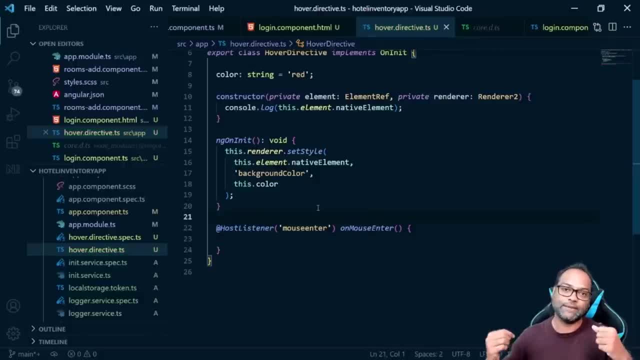 host listener, so host listeners are host listener, so host listeners are actually used to listen to any event actually used to listen to, any event actually used to listen to any event which is happening on your parent, which is happening on your parent, which is happening on your parent. component. 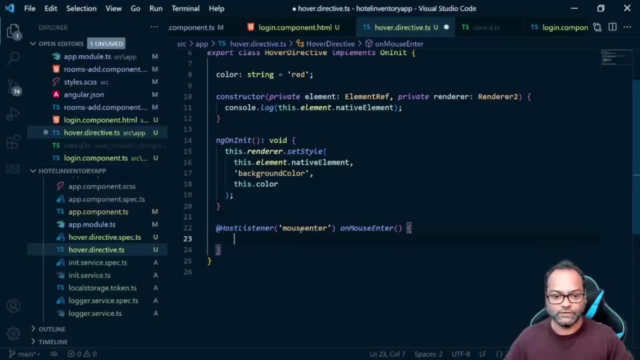 component, component, the component where this particular, the component where this particular, the component where this particular directive is applied. so let's see directive is applied. so let's see directive is applied. so let's see what we can do here. so here i'll just what we can do here. so here i'll just 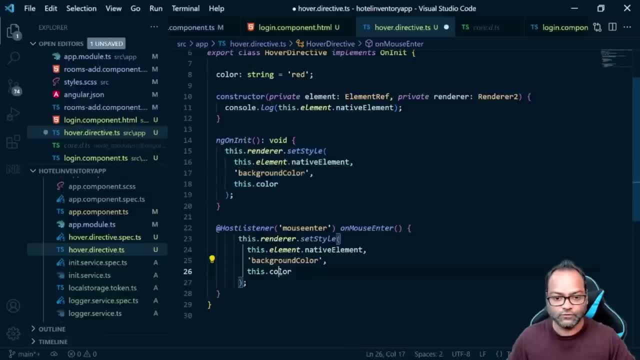 what we can do here. so here i'll just copy the same, copy the same, copy the same, and i'll say okay whenever we hover, and i'll say okay whenever we hover, and i'll say okay whenever we hover. change the background color to green. change the background color to green. 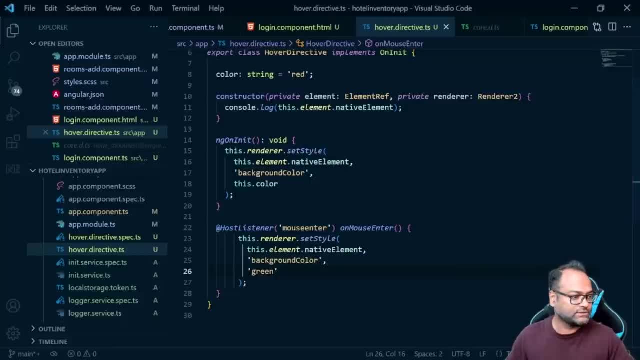 change the background color to green. so on, mouse enter my background color. so on, mouse enter my background color. so on, mouse enter my background color will be changed to green. will be changed to green. will be changed to green. let's, let's, let's, go ahead and verify and you can see on. 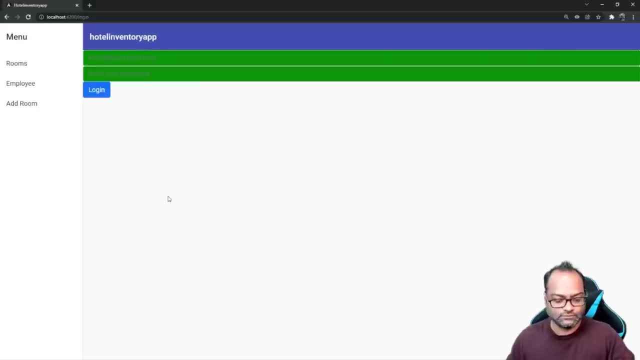 go ahead and verify and you can see on: go ahead and verify and you can see: on hover, let's refresh it again, hover, let's refresh it again, hover, let's refresh it again, and and and refresh it again. and on hover the background color is: refresh it again. and on hover the background color is: 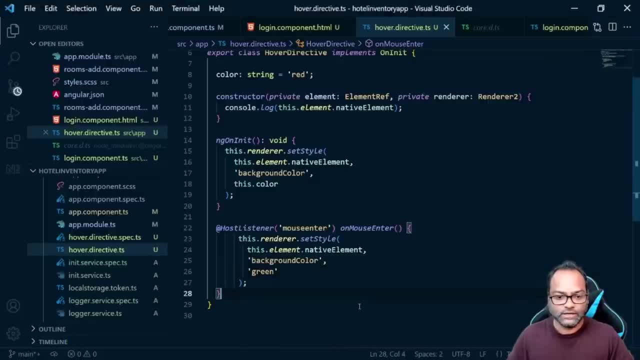 refresh it again and on hover, the background color is changed to green, changed to green, changed to green. similarly, we can, similarly we can. similarly we can listen to mouse leave event so we can say: listen to mouse leave event. so we can say: listen to mouse leave event. so we can say: okay, on mouse leave, just go ahead. and 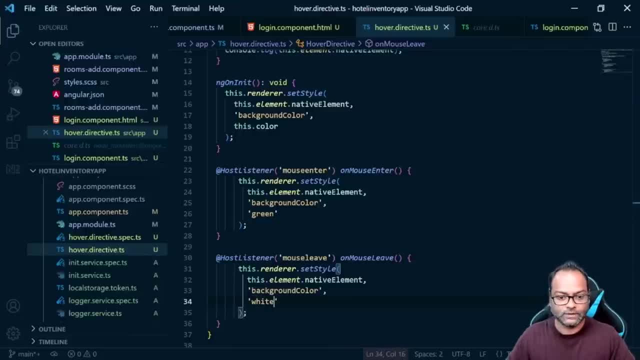 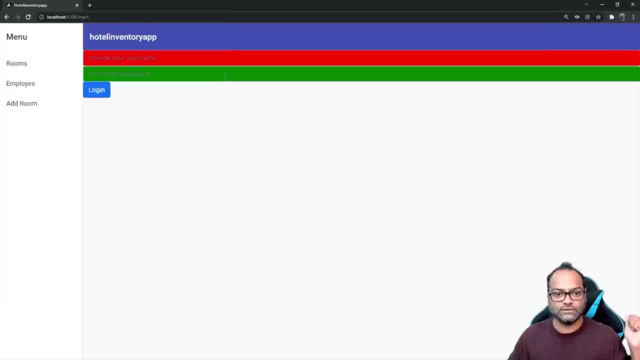 okay on mouse leave, just go ahead. and okay on mouse leave, just go ahead and make this to white. so as soon as i leave, it becomes white. so as soon as i leave, it becomes white. so as soon as i leave, it becomes white. so you can see, i can actually go ahead. 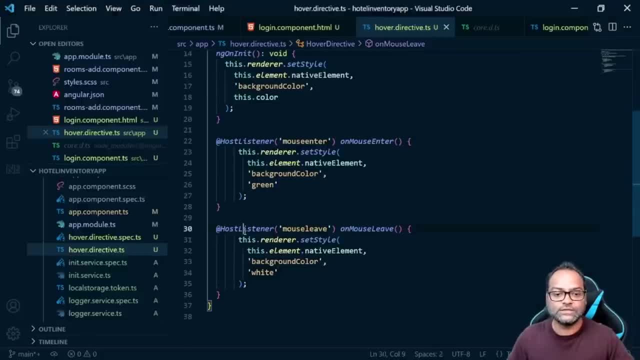 so you can see i can actually go ahead. so you can see i can actually go ahead and do that as well by using the host. and do that as well by using the host. and do that as well by using the host listener. so host listener will listen to. 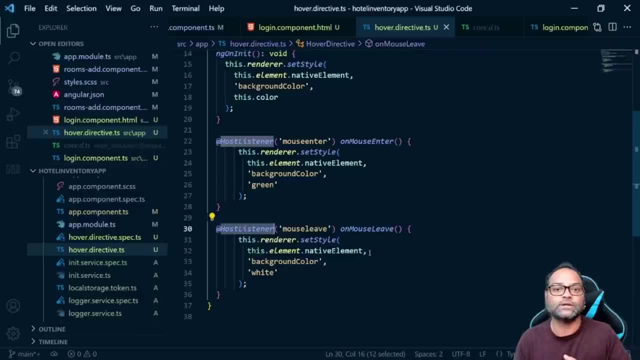 listener, so host listener will listen to listener, so host listener will listen to any event which is happening on the, any event which is happening on the any event which is happening on the component where this particular directive, component, where this particular directive component, where this particular directive is applied. 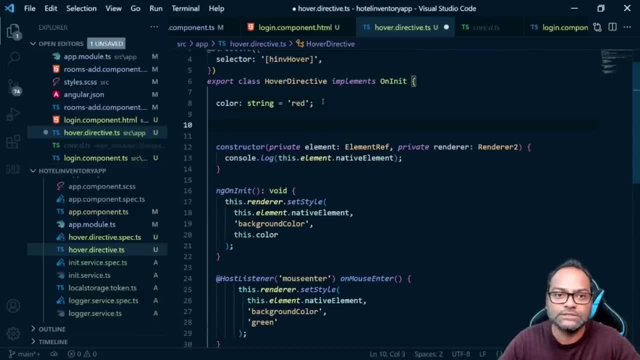 is applied, is applied. what else, so you can also pass the what else? so you can also pass the what else? so you can also pass the properties properties properties, input properties, input properties, input properties to your directives as well as output to your directives, as well as output. 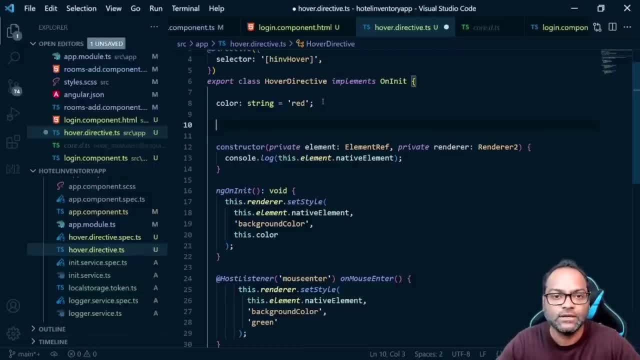 to your directives, as well as output properties, because, as i said, properties, because, as i said properties, because, as i said, it's same right, i mean, uh, it's same right. i mean uh, it's same right. i mean uh, the only difference is it doesn't have a. 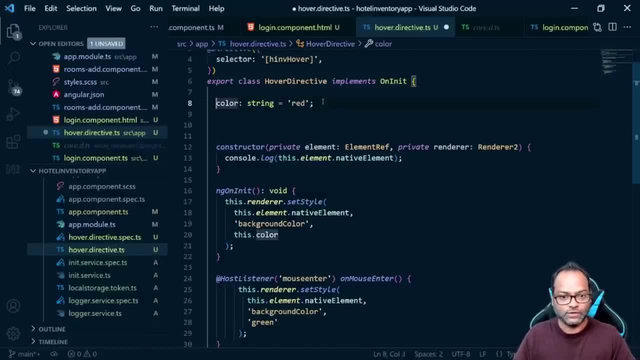 the only difference is it doesn't have a. the only difference is it doesn't have a template to deal with, template to deal with, template to deal with. so here let's try to convert this. so here let's try to convert this. so here let's try to convert this color. 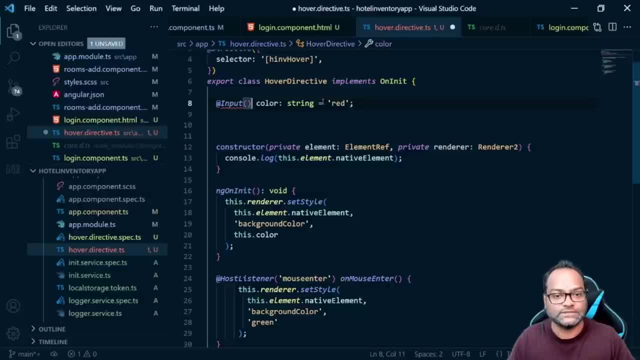 color, color. so now the user or developer can decide. so now the user or developer can decide. so now the user or developer can decide which color to pass. so i'll say okay, which color to pass, so i'll say okay, which color to pass? so i'll say okay, this is now input. 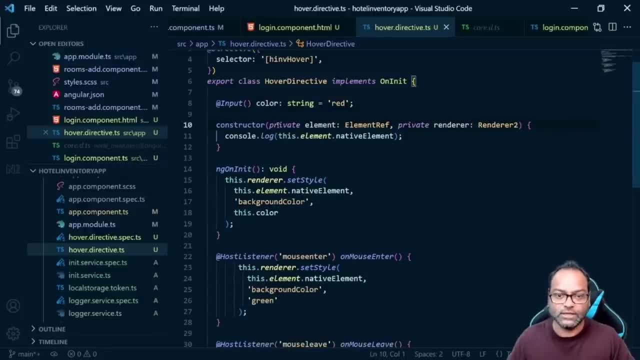 this is now input. this is now input which is of type color and by default it's which is of type color and by default it's which is of type color and by default it's red in case someone does not pass it. red in case someone does not pass it. 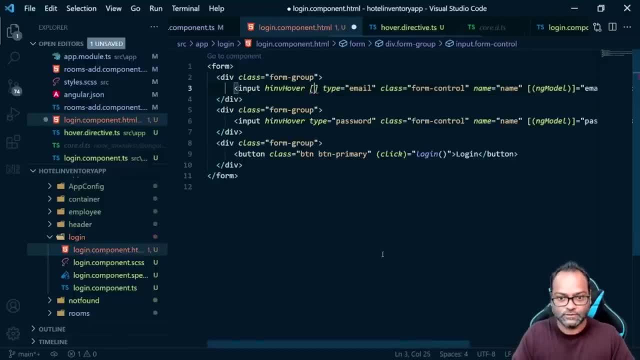 red, in case someone does not pass it, if i pass it. so let's say this is input: oh sorry, this is color we can actually. oh sorry, this is color, we can actually. oh sorry, this is color, we can actually. just avoid this. just avoid this, just avoid this box property. i can say: color equals to. 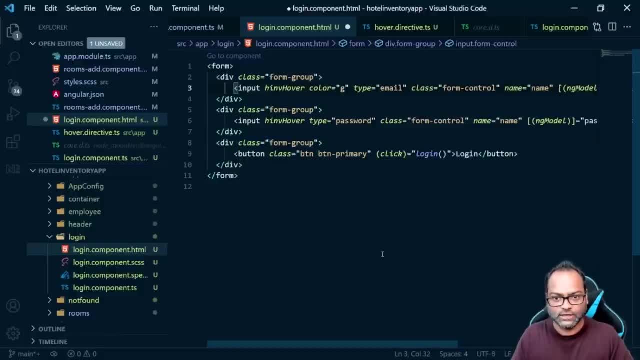 box property, i can say: color equals to box property, i can say color equals to, and because, uh, this is going to be a, and because, uh, this is going to be a, and because, uh, this is going to be a string only, string only, string only. so i can say, okay, uh, for this, just use. 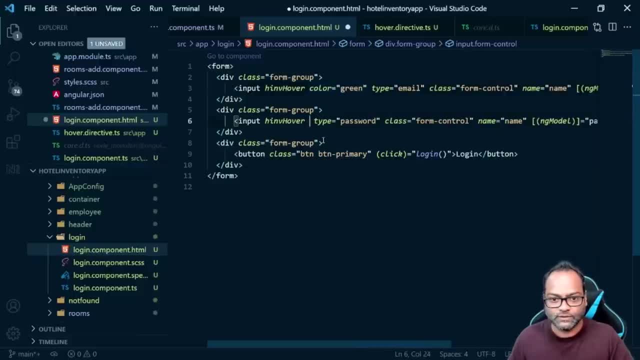 so i can say okay, uh, for this just use. so i can say okay, uh, for this just use. color is equals to green, color is equals to green, color is equals to green. and for this, uh, use steel blue another. and for this, uh, use steel blue another. 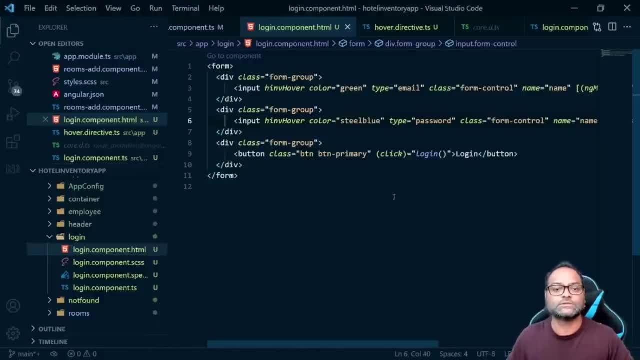 and for this uh use steel blue, another, my, my, my, one of my favorite colors, one of my favorite colors, one of my favorite colors. so let's see, and here it is, so you can see, uh, let's, and here it is, so you can see, uh, let's. 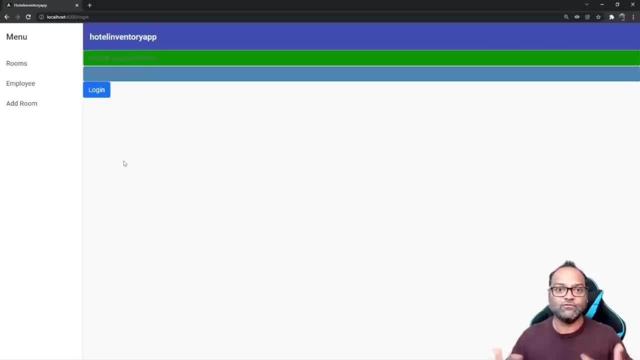 and here it is. so you can see, uh, let's refresh it again, refresh it again, refresh it again. so now we are, we are able to pass the. so now we are, we are able to pass the. so now we are, we are able to pass the default color to. 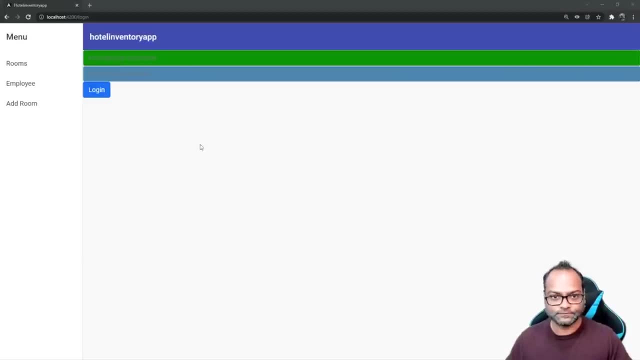 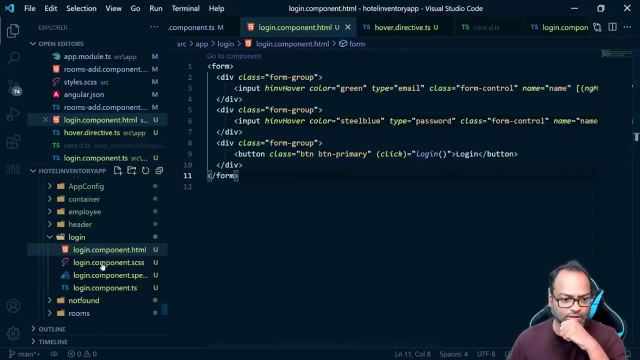 default color, to default color to your directive, your directive, your directive by using, by using, by using the uh, the uh, the uh, by making the input as a input property, by making the input as a input property, by making the input as a input property, what else we can achieve? 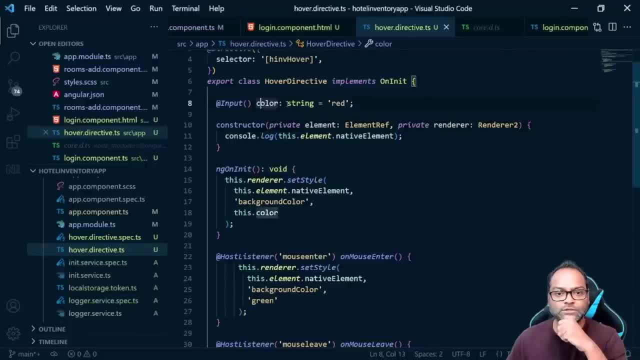 what else we can achieve, what else we can achieve. i'll show you one more thing which can. i'll show you one more thing which can. i'll show you one more thing which can be done, be done. so is it possible that i can just combine. so is it possible that i can just combine. 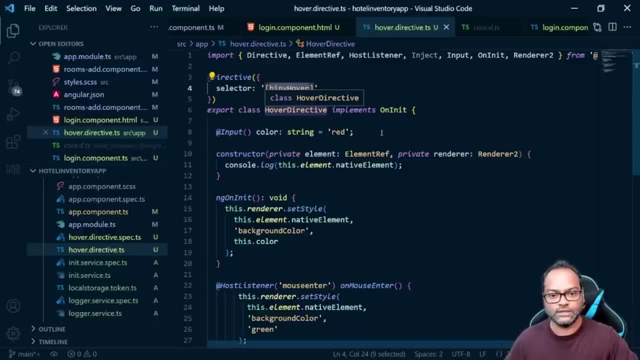 so is it possible that i can just combine my input properties with my selector as my input properties with my selector, as my input properties with my selector as well? well, well, how let's do that? so how let's do that? so how let's do that? so there are multiple ways. i'll- uh, you can. 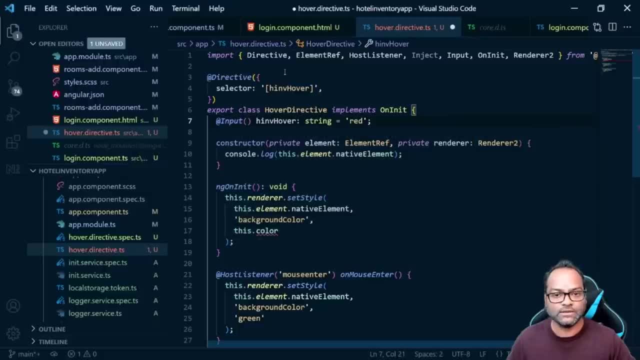 there are multiple ways i'll- uh, you can. there are multiple ways i'll, uh, you can actually just do, actually just do, actually just do. by using this so you can keep your input by using this, so you can keep your input. by using this, so you can keep your input name and same as your selector. 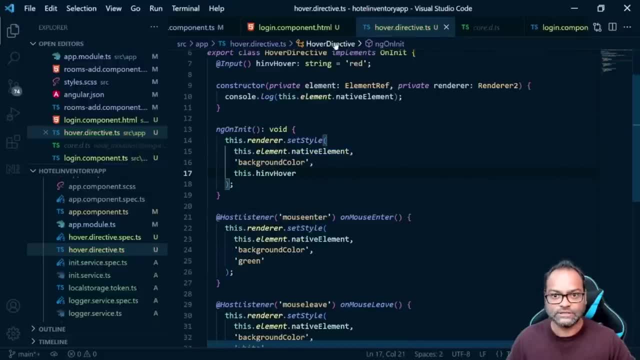 name and same as your selector name, and same as your selector, and let's change this, and, and let's change this, and and let's change this. and once it is done here, we will go to this. once it is done here, we will go to this. once it is done here, we will go to this and now. 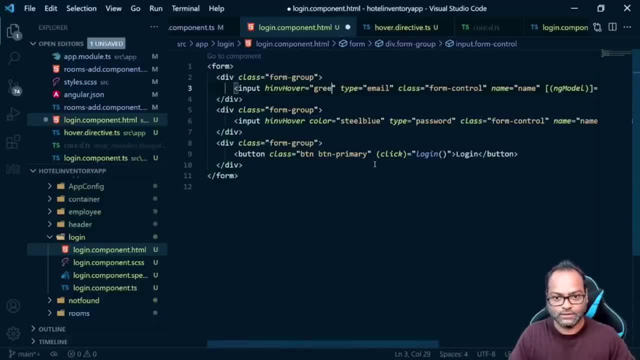 and now, and now i'll say h, green, green, green, and, and, and same here. so i'll say, okay, this is same here. so i'll say, okay, this is same here. so i'll say, okay, this is equals to equals to equals to still blue. let's see. 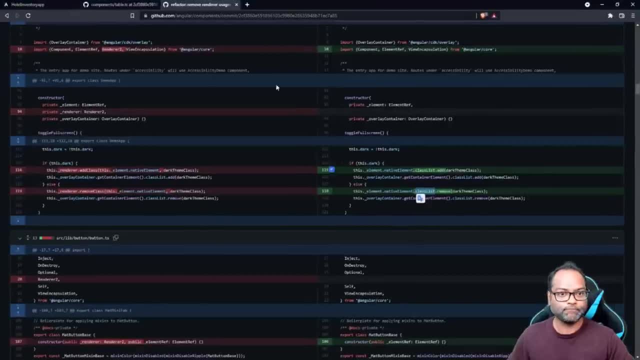 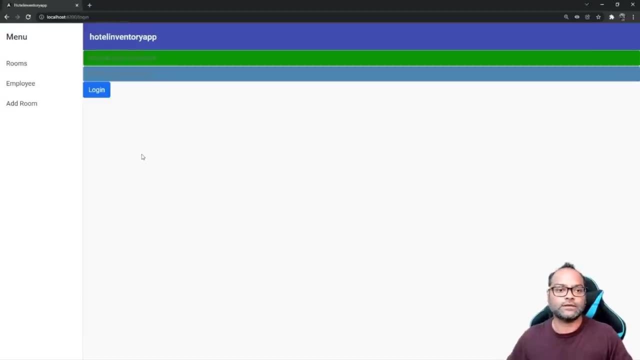 still blue. let's see still blue, let's see if it works. you can see uh still works right, so we. you can see uh still works right, so we. you can see uh still works right. so we are now uh, what we have uh done is. are now, uh, what we have uh done is. 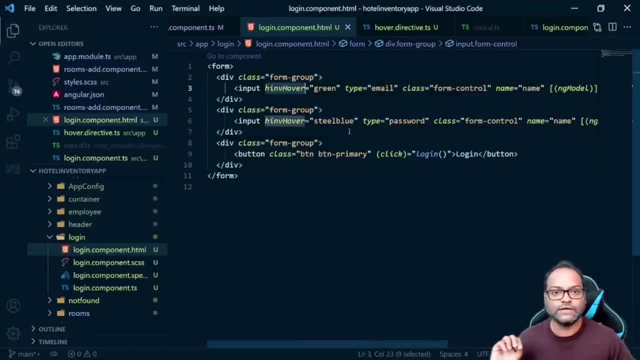 are now, uh, what we have uh done is now we are not using any extra variable. so now we are not using any extra variable. so now we are not using any extra variable. so we are, we are using the same variable. we are, we are using the same variable. 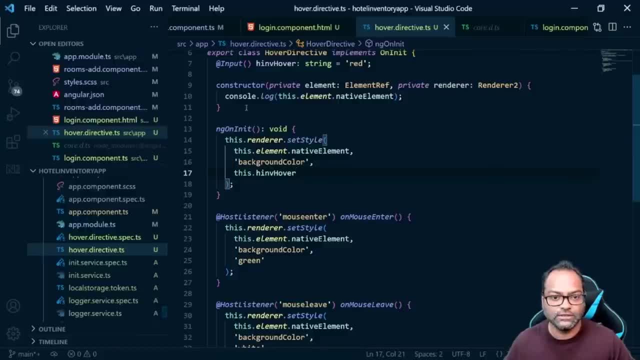 we are. we are using the same variable name- name, name- to actually capture the color as well by to actually capture the color as well, by to actually capture the color as well, by using the same input property as of my, using the same input property as of my. 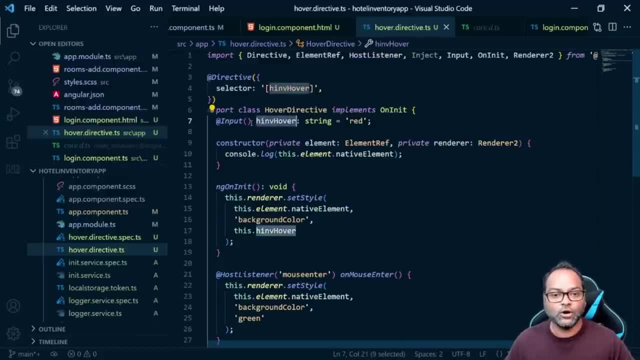 using the same input property as of my selector property. this is something selector property, this is something selector property. this is something which can be achieved, which can be achieved, which can be achieved. so, or there, i mean, there is another hack. so, or there, i mean, there is another hack. 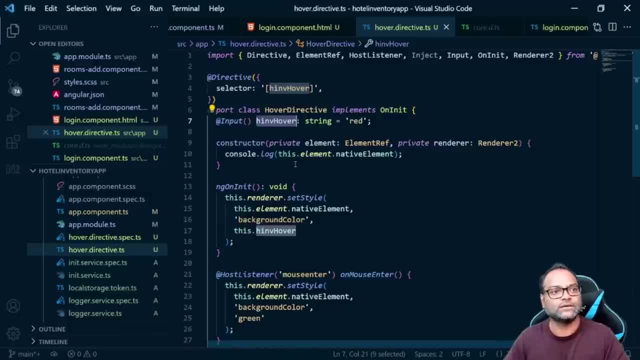 so, or there, i mean there is another hack, but i will not tell you because. but i will not tell you because, but i will not tell you because that's uh what you can say. that's a. that's uh what you can say. that's a. that's uh what you can say. that's a linting error. 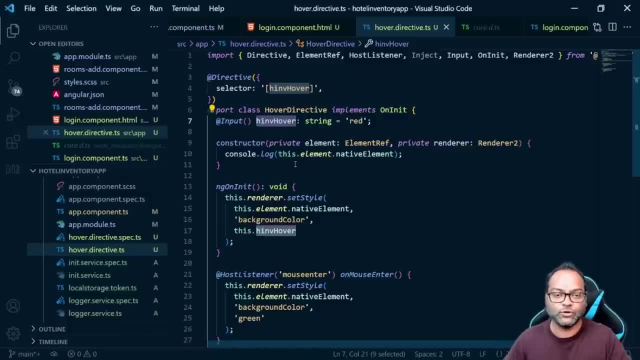 linting error. linting error: uh in most of the application. that's a uh in most of the application. that's a uh in most of the application. that's a lending error. you should not do it. lending error. you should not do it. lending error, you should not do it. but yeah, so this is. this is another. 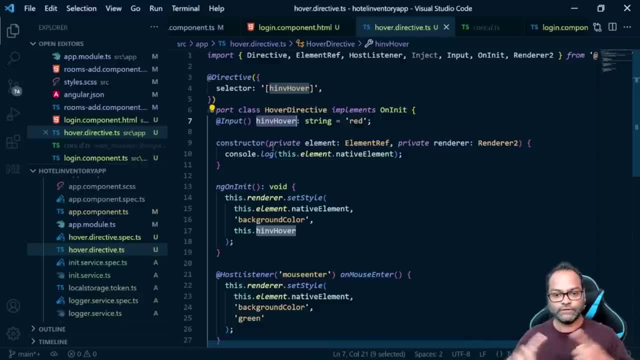 but yeah, so this is, this is another. but yeah, so this is, this is another example how you can actually deal with example, how you can actually deal with example, how you can actually deal with directives. so what we did here is we directives. so what we did here is we. 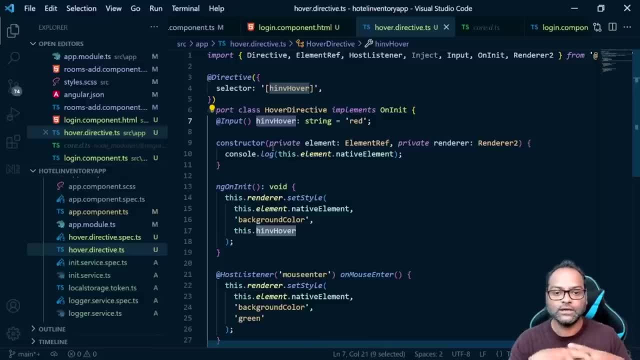 directives. so what we did here is: we created a directive, we applied the created a directive, we applied the created a directive. we applied the directive to our components directive to our components directive to our components, and we discussed about element ref and we discussed about element ref and we discussed about element ref. renderer to. 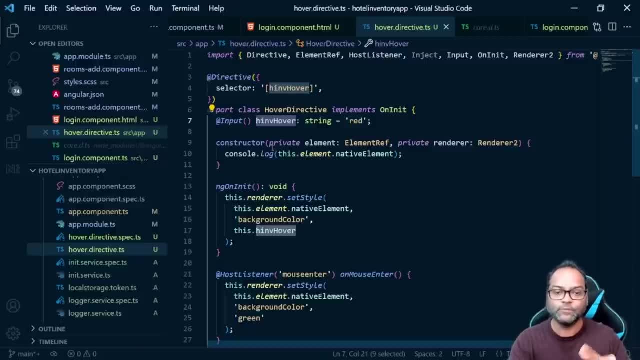 renderer to renderer to the apis which you can use to change the, the apis which you can use to change the, the apis which you can use to change the behavior of your dom. then we discuss behavior of your dom. then we discuss behavior of your dom, then we discuss about host listener, how you can actually 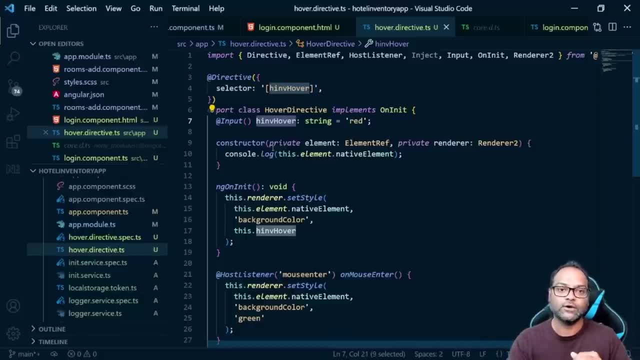 about host listener, how you can actually about host listener, how you can actually listen to any event which is happening. listen to any event which is happening. listen to any event which is happening on your components, where your directive on your components, where your directive on your components, where your directive is applied. so directives are some uh. 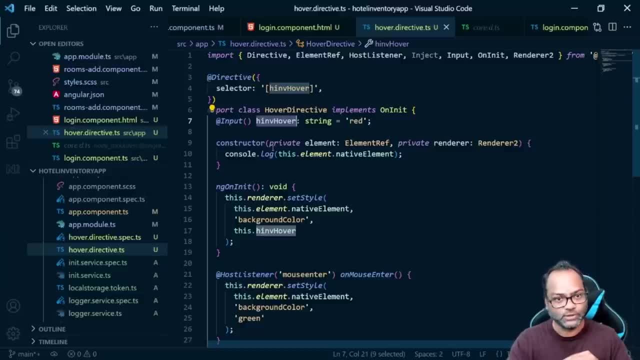 is applied, so directives are some. uh is applied, so directives are some. uh, what? what directive is it's a helper? what? what directive is it's a helper? what, what directive is it's a helper? function for your components? or for function for your components, or for function for your components or for any dom element? 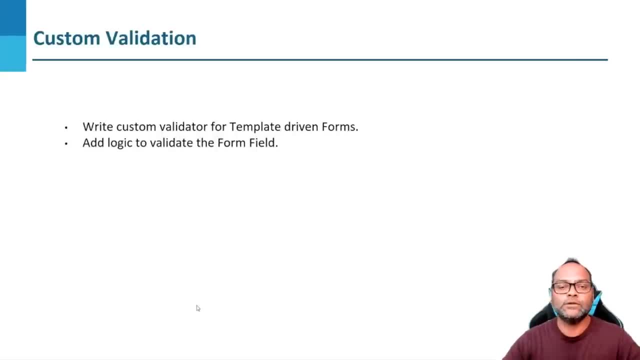 any dom element, any dom element. so in this video, we will see how we can. in this video, we will see how we can. in this video, we will see how we can utilize, utilize, utilize the custom uh directives to create a. the custom uh directives to create a. 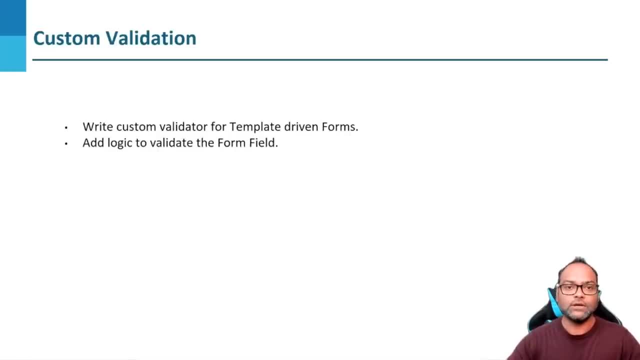 the custom uh directives to create a custom validator for your components. custom validator for your components, custom validator for your components. this uh, this uh, this uh technique can be applied on any template technique can be applied on any template technique can be applied on any template driven forms. 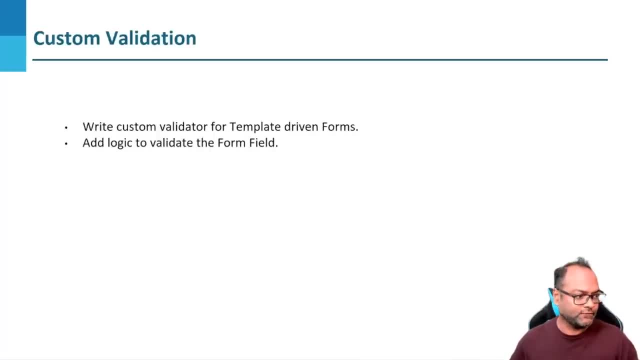 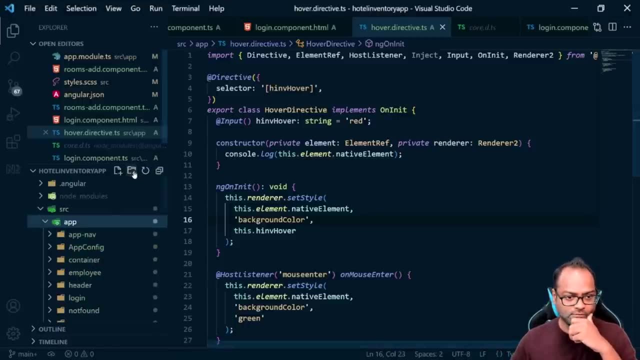 driven forms. driven forms. so let's go ahead and do that. so first we. so let's go ahead and do that. so first we. so let's go ahead and do that. so first we will create a directive. so i'll create, so i'll create, so i'll create folder. 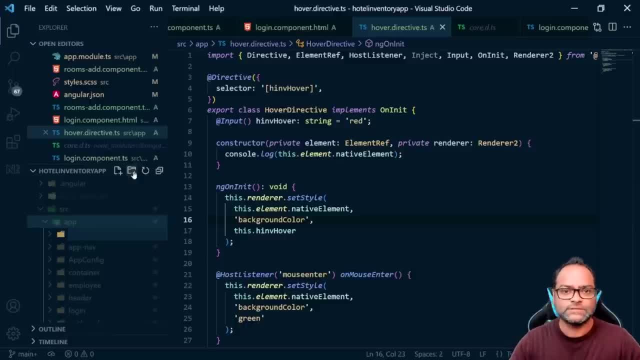 folder folder, and let's create an email validator so, and let's create an email validator so, and let's create an email validator. so, as we said, our username is email. so if, as we said, our username is email, so if, as we said, our username is email, so if we detect a. 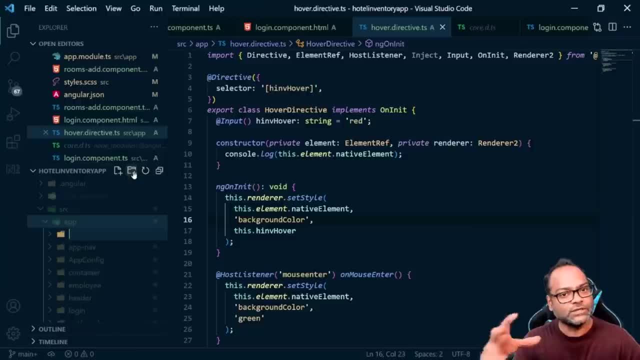 we detect a, we detect a text called test in the email. we will say text called test in the email. we will say text called test in the email. we will say, okay, this user is not valid user. so okay, this user is not valid user. so okay, this user is not valid user. so let's see, i'll call it as email. 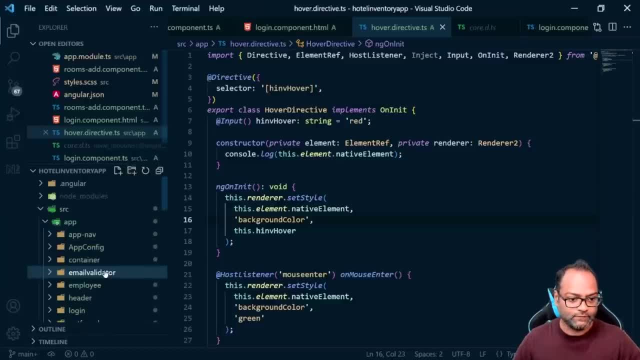 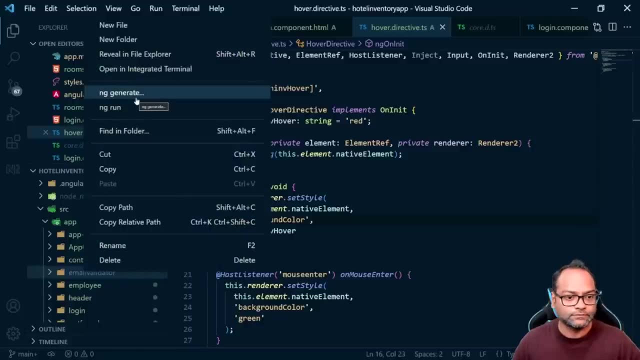 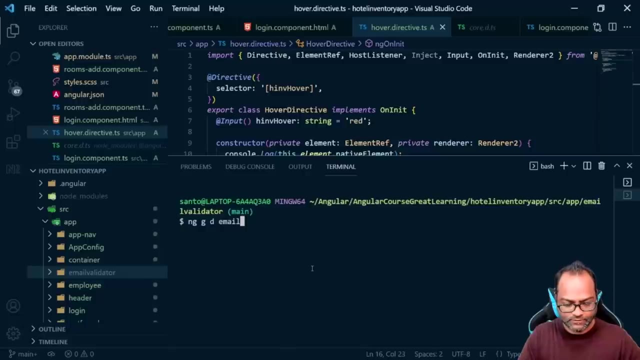 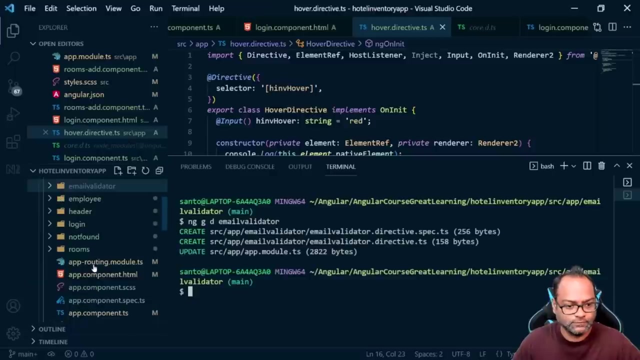 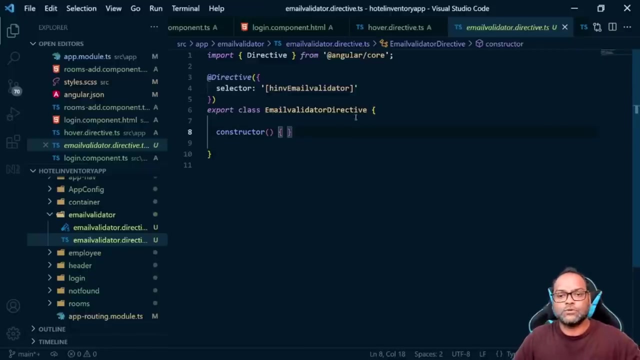 let's see, i'll call it as email. let's see, i'll call it as email validator. validator- sorry, how to add this, so remember so in case, how to add this, so remember so in case. how to add this, so remember so in case you are trying. 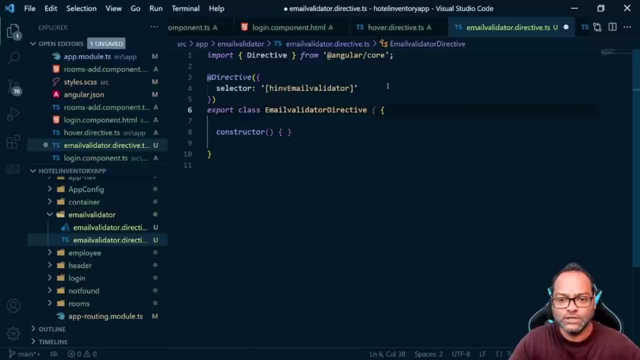 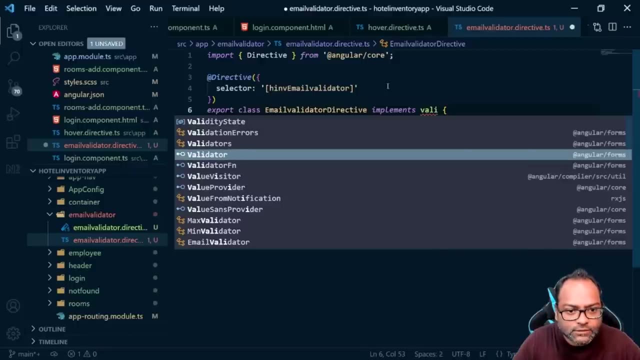 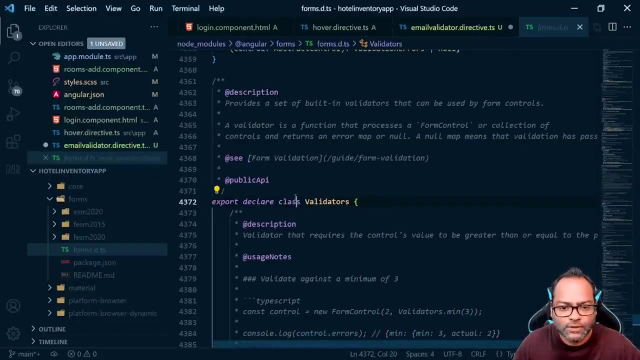 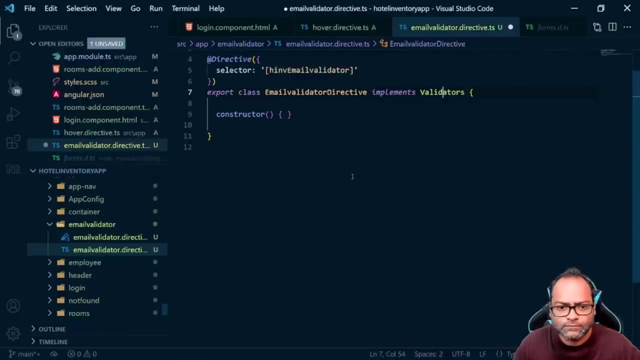 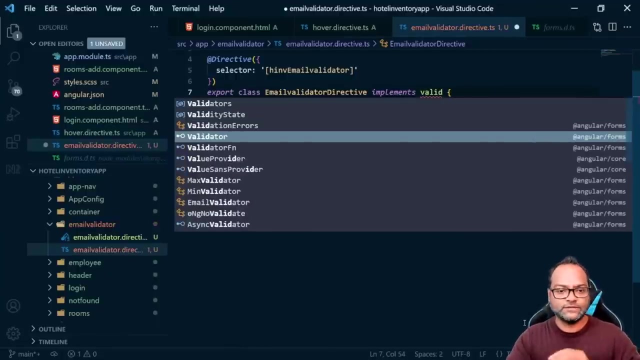 you are trying to implement a custom validator for your template driven forms, you have to implement something known as a validator. it should be. it's a class, so it should be extend. there are two things. so let me just tell you. so there is an interface validator which will be used. 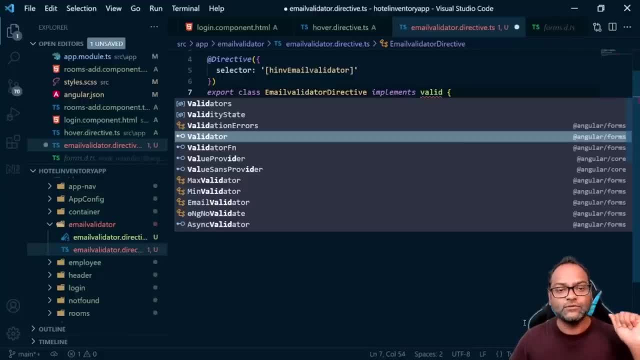 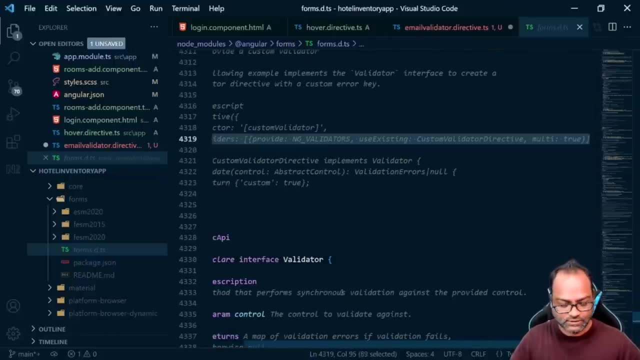 for our use case. there is a class called validators, Which we will use with reactive forms. So let's implement validator and see what we need to do. So we have to add something like this: I'll just copy this and then we'll talk about it. 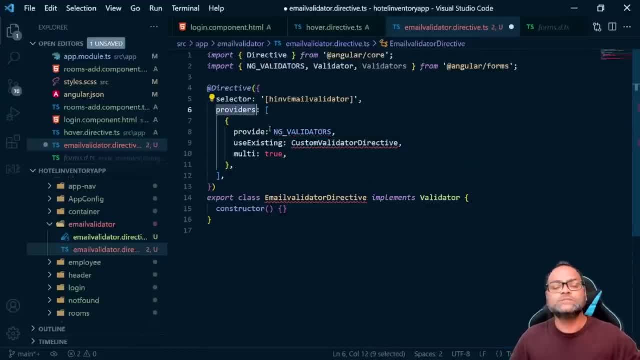 So here you can see, I'm adding a providers and we are saying: provide ng validators, use existing, where you will provide this class and then you will say multi: true, What is the purpose? Let's, we'll talk about it. And this validator class actually gives you a validate method. 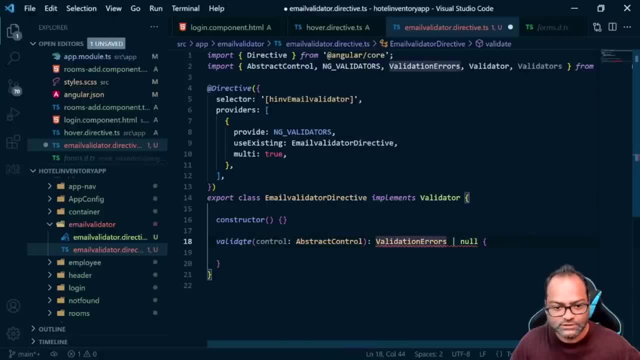 Which has signature like this. So it gives you control validation errors. So this is the interface, right? So this is the function which is provided by interface. Let's talk from top to bottom what we have done Angular already has, like all the built-in validators, right. 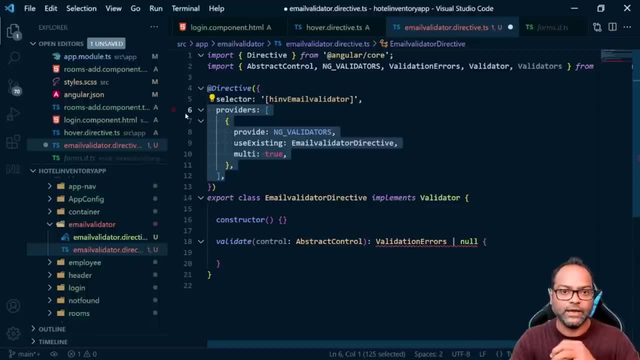 Which we have seen email required and patterns everything. In case we want to actually add our own validator, we have to actually let angular know that we are adding our own validator By using an Uh Injection token. remember we did it for HTTP interceptor. 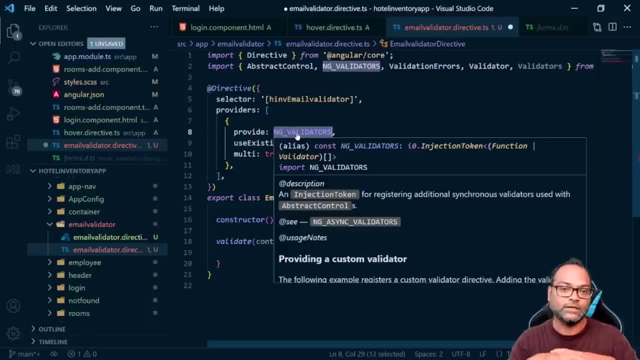 We added our HTTP interceptor as part of the angular's interceptor queue. So similarly here what we are doing is we are adding our validator into all the existing validator which exists, And for that we are saying: whenever I try to use this particular selector, you have. 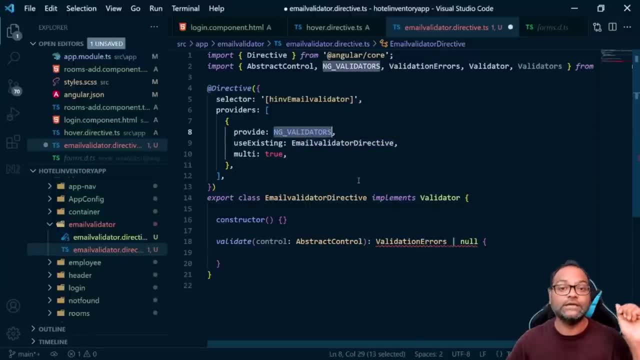 to go ahead and add this particular class as part of the validators which exists. That's why we are saying multi: true, because it's not a object, it's an array. It's an array of All the validators which exists. now, here you can see. it returns with a null or validation. 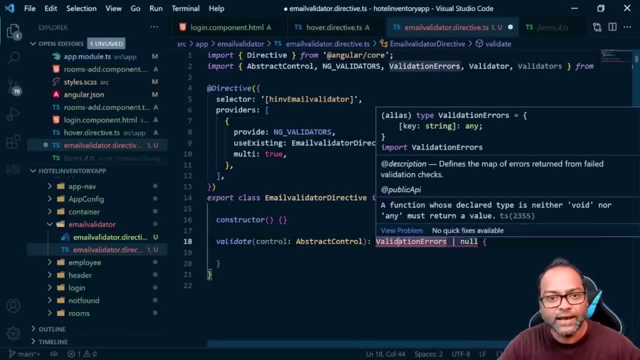 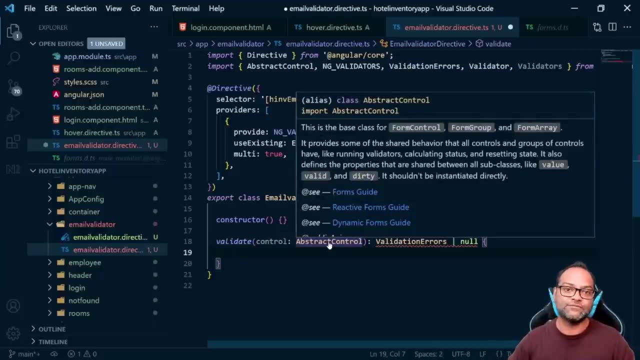 errors. Validation errors is type of key and value. So here we can do something like this: This abstract control actually gives you the value of the control. This is base class for most of the classes related to forms. Remember this one thing: there is no difference between template driven and reactive forms. 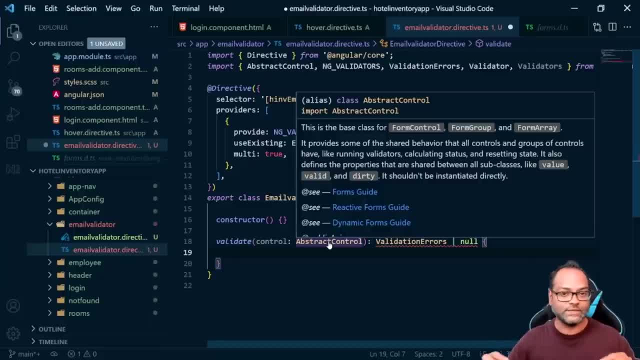 right, Because the APIs are same, So the core APIs are same. It's the only way. Uh, The flavor changes, right? I mean we. what we have seen till now is template driven form where we did everything on HTML. 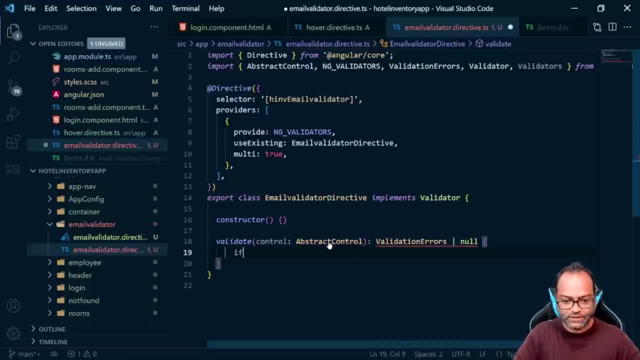 We will see the form and you will know the difference. but right here we'll do something like this. We'll say control And as as uh, this is a input control. So I'll say, okay, if this uh control dot value. now you can see, I'm not able to get. 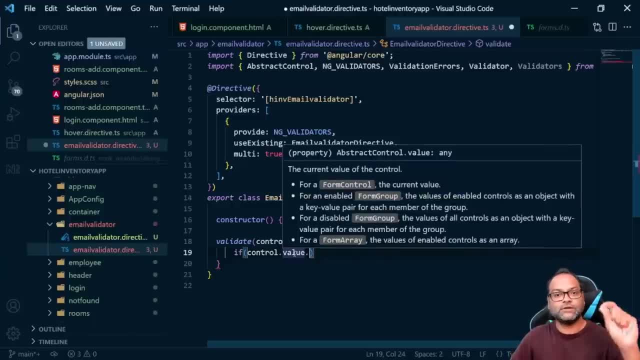 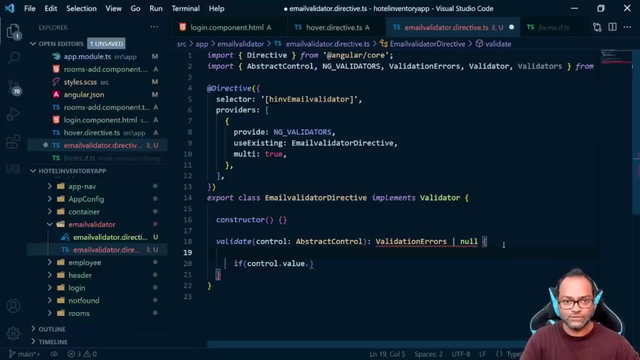 anything after this. Why So? so if you see the value is type of any, if I need uh, or if you want to, you can type it. If you want the typings, I'll say just doing this So you can actually do the control dot value. 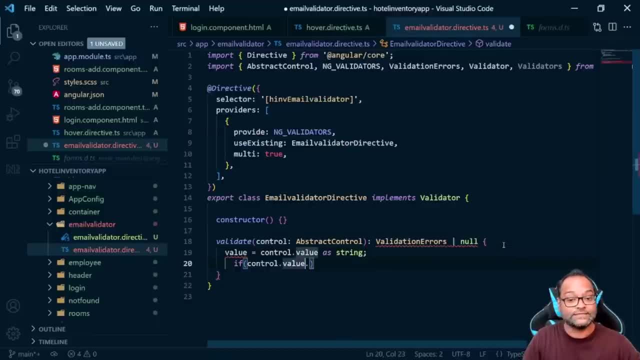 As we know that we are going to get string, just typecast it as string And now we can do something like this: Value dot. Now you can see. uh, I'll say okay. if it includes the word test, I will find it. 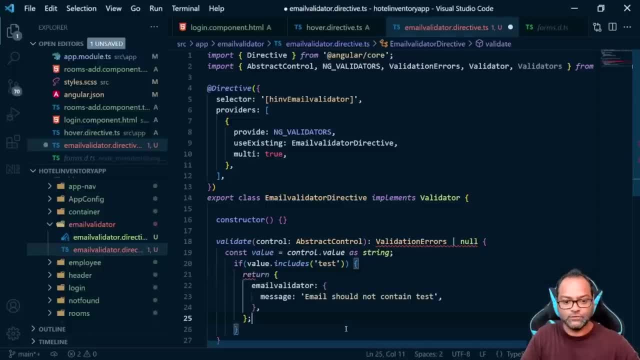 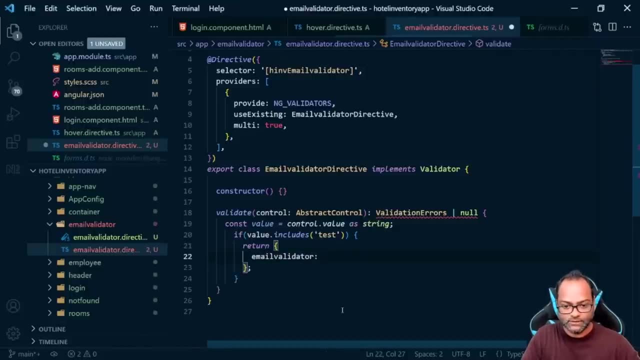 Okay, I will return. So this is how you will return: an email validator. So you'll say email validator, and then it's key value. So I can say, uh, email, uh, valid email, uh, right, And so let's say invalid email too. 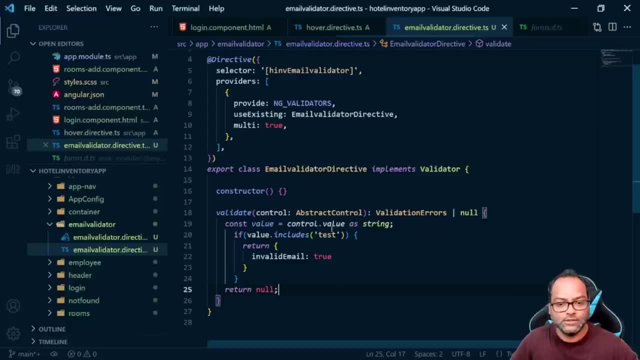 And if there is no error, it means we can return null. So you can see the uh typing error is gone here And let's apply this validator now to email and see if we get the uh error we are looking at. 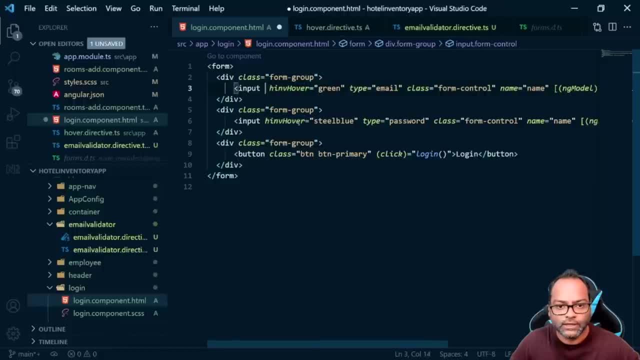 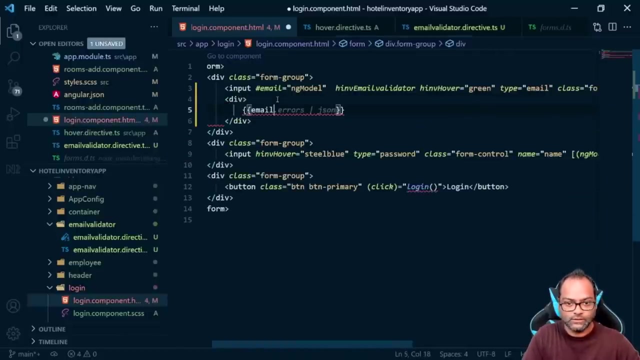 So now let's go back to login component. apply this to this one And I. we will take hashtag email. uh equals to ng model, right? So we have seen how to get the access to this particular control. Okay, So let's go ahead and verify the code. 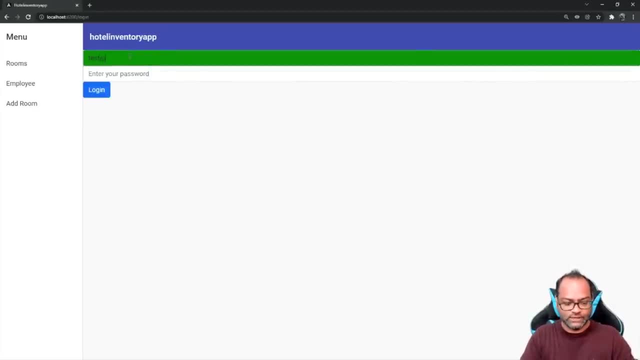 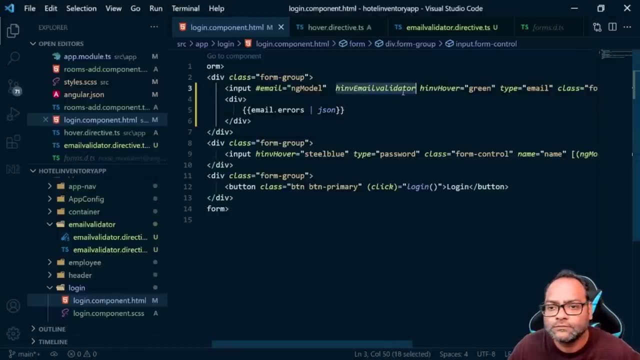 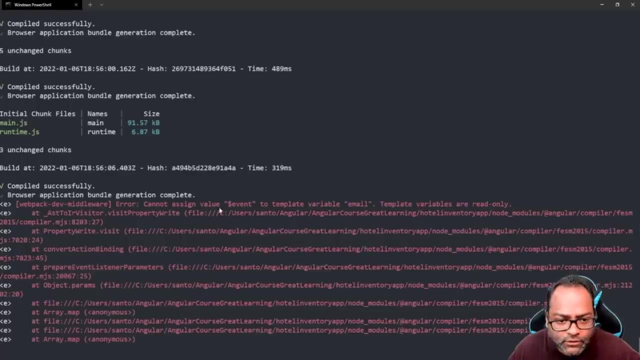 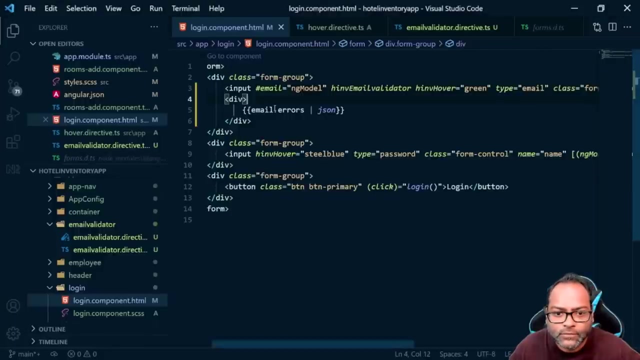 Now we have this. uh, I'll stop type test at the rate. gmailcom. Let's see. ah, there's some errors. cannot assign value variable. email template variable are read only where I'm trying to assign a value email dot. errors in email. 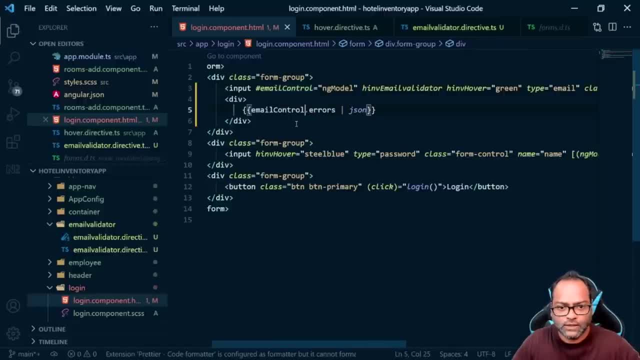 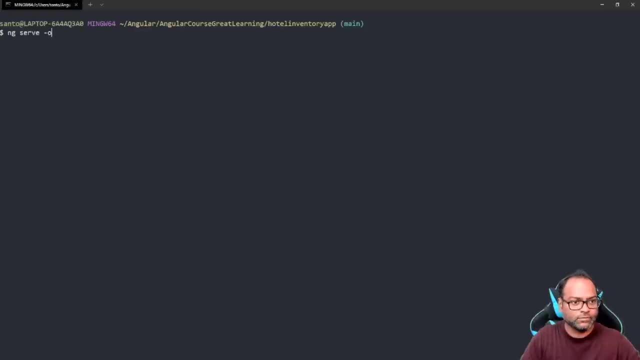 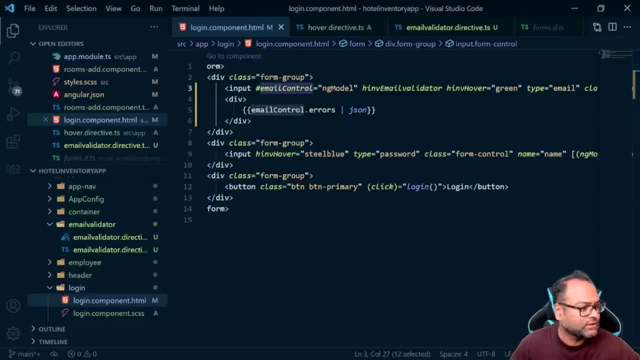 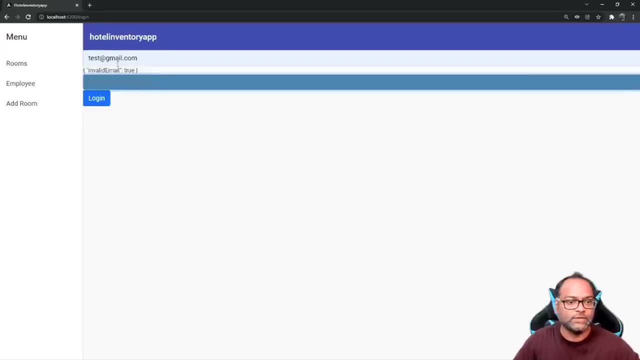 Let's verify it again. So I'm saying email control, because probably I said email, that's why it crashed, But it's, it's verified. Yeah, So now we have null, so it means it's valid. So I'll say: test at gmailcom and you can see invalid email too. 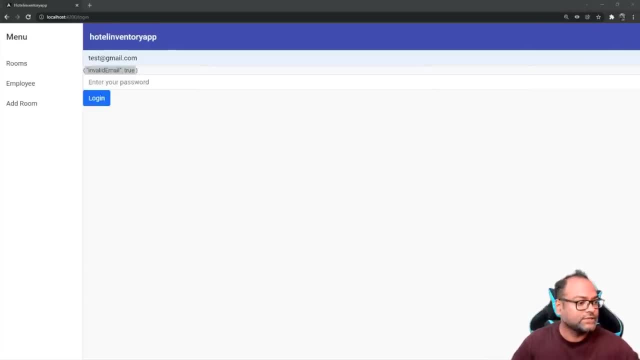 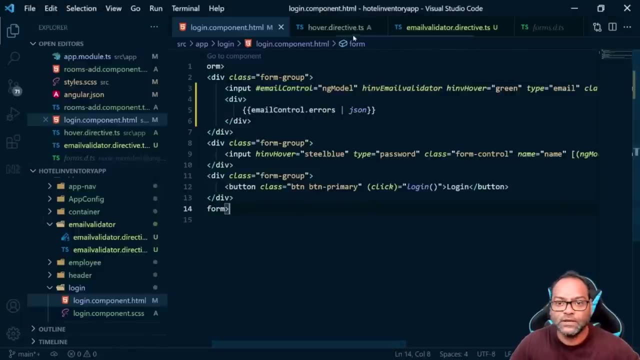 So we have the validation error available here, And what we just did is we added our custom validation to this particular control by using a custom directive, and now you can just go ahead and add this validator. it is reusable, right? so you can actually go ahead and use this custom directive anywhere you want within your application. 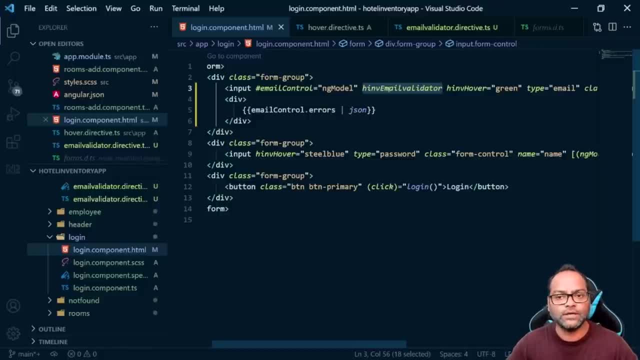 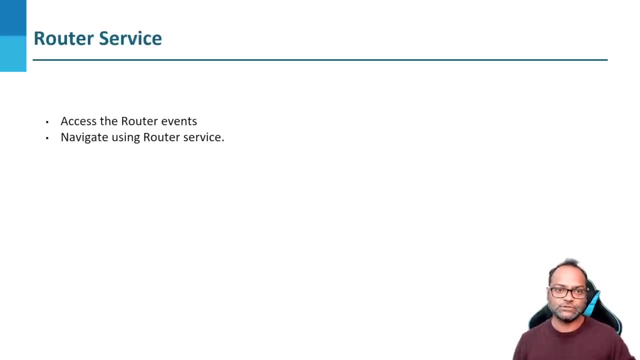 and this is it from the custom writing: your own validator using custom directive. now we are back to the routing part. remember i said we will create some views using template driven forms and and then we'll be back to the routing and the place where we left is. 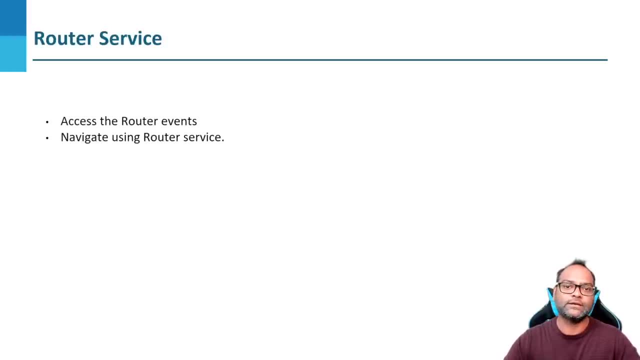 router service. so let's go ahead and see an example how we can actually use router service and a small example. so far we have done some navigation right, so we have used router link to navigate and we have used router link to navigate and we have used router link to. 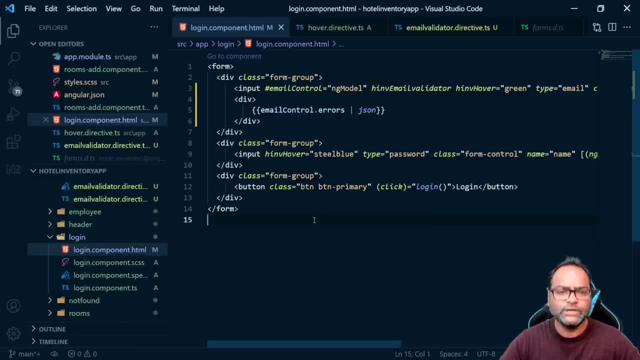 to whatever view we want to. But in case we want to do it programmatically, it means, let's say, we have some logic and after that logic is satisfied we want to navigate to some other view. That's why we created Login Component. 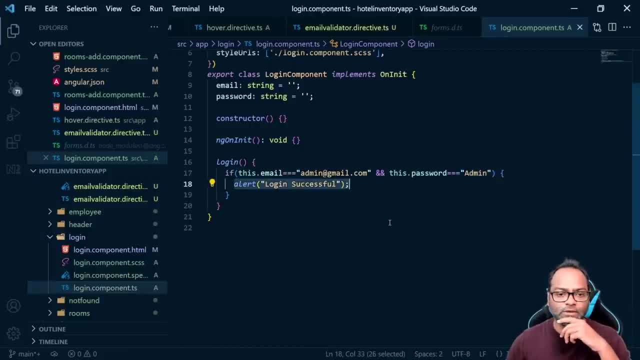 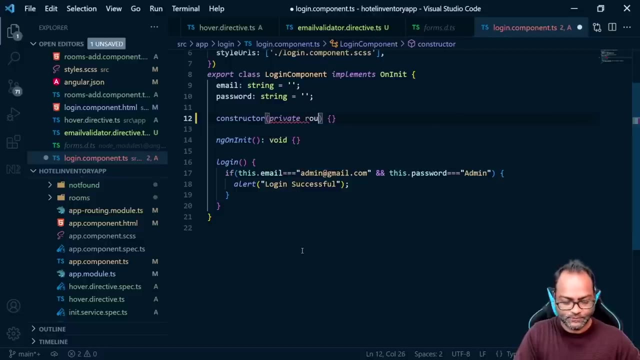 So remember we just added this alert login successful. But in case I want to redirect to rooms after we are logged in, how we will do that. So Angular has a service called Router, So let's go ahead and see. We'll use Route, which is type of Router. 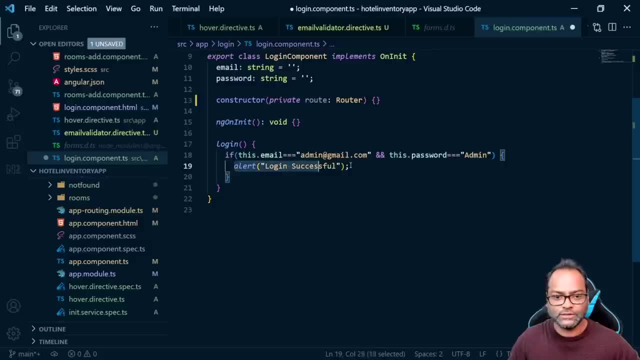 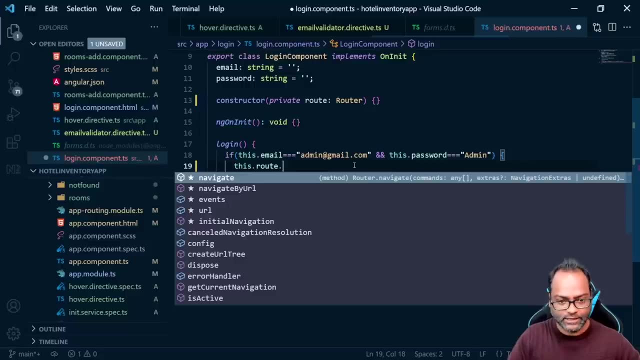 And it comes from Angular slash Router. so you can see this. And now let's see how we can navigate. There are many methods which this particular API exposes, So I'll say Routedot And we will be using Navigate. So in Navigate you can just pass the URL. 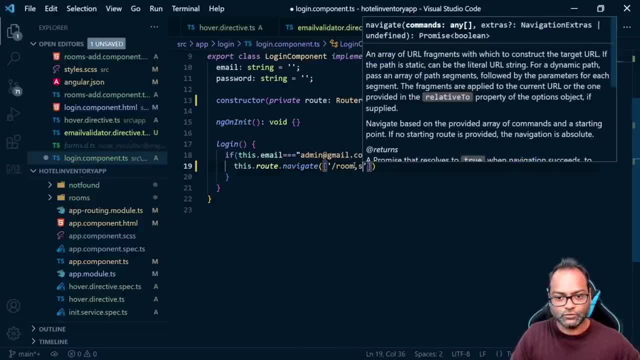 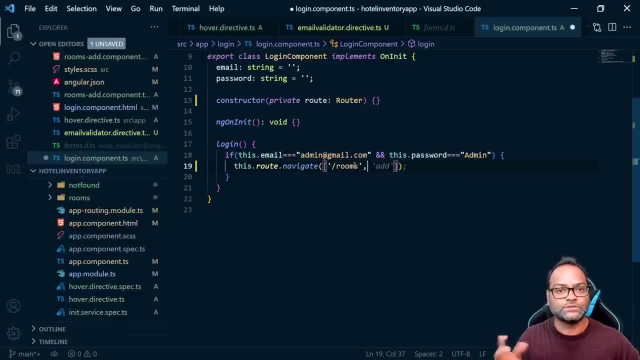 where you want to redirect. So I can say: I want to redirect to rooms, And the thing is you can pass the command as well. So, for example, if I want to say a room slash ad, I can do something like this. 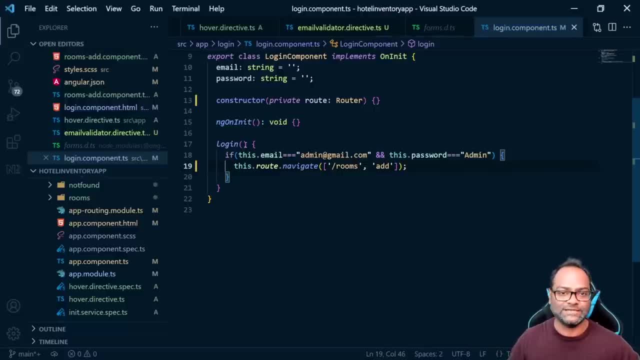 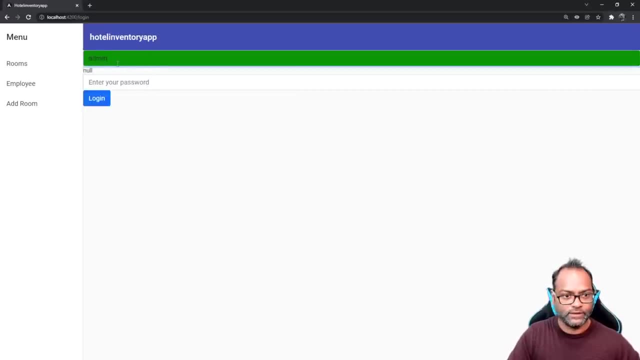 Let's try this out. We already have a URL called room slash ad, So let's provide admin at gmailcom And this will be admin. So and let's click on Login And you can see we are redirected to rooms slash ad. 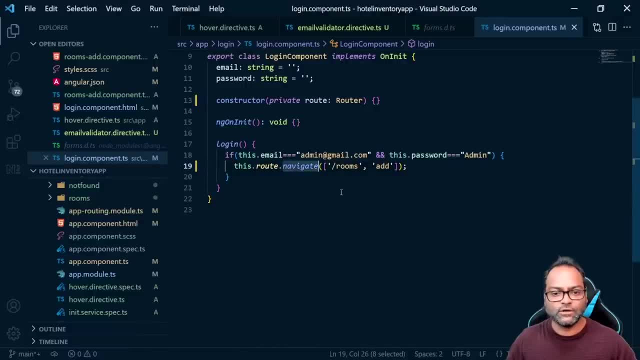 So this is how you can do it programmatically. There is another API called Navigate by URL as well, So you can see, in this case you can just give the URL, So you can say: it will be slash rooms, slash ad, And let's see. 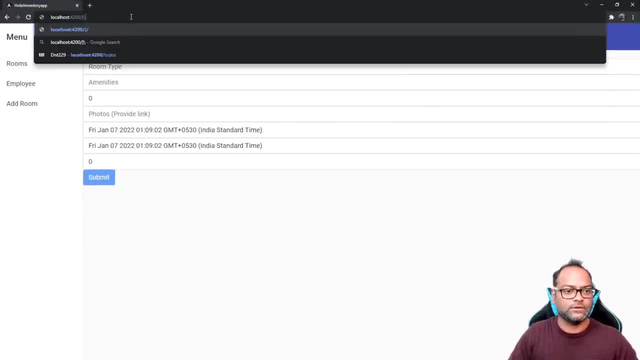 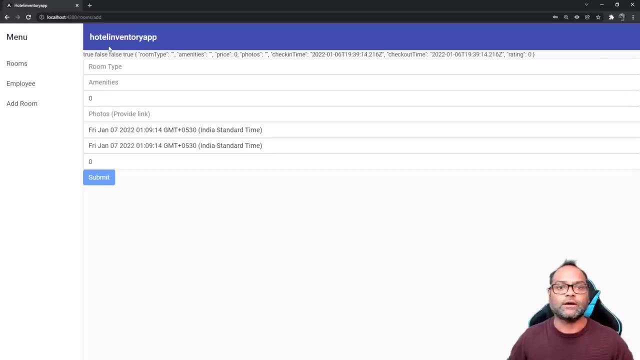 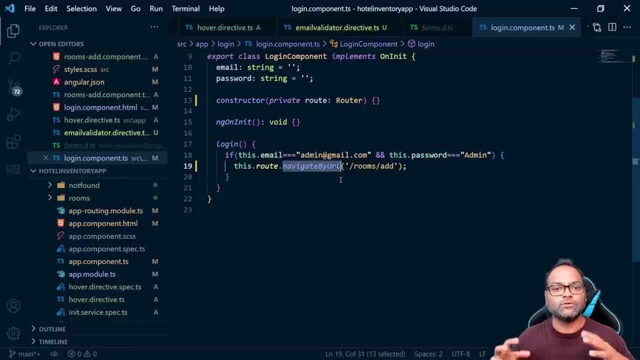 Let's remove this and go back to the login page. Now we are back to the rooms slash ad. So the only thing is the difference is between Navigate by URL and Navigate is. Navigate by URL will take the list of commands, So whatever you are passing inside, 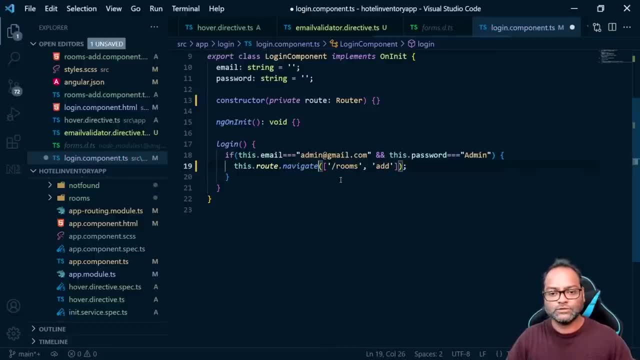 So let's go back to Navigate. So here we are passing the list of actions, or you can say commands, And Navigate method will create the entire URL for us. In Navigate by URL we are saying, OK, this is the URL. 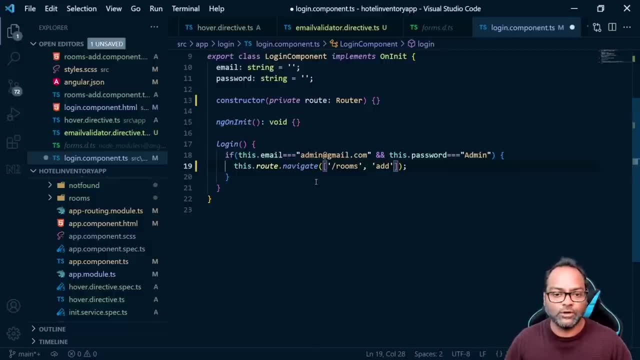 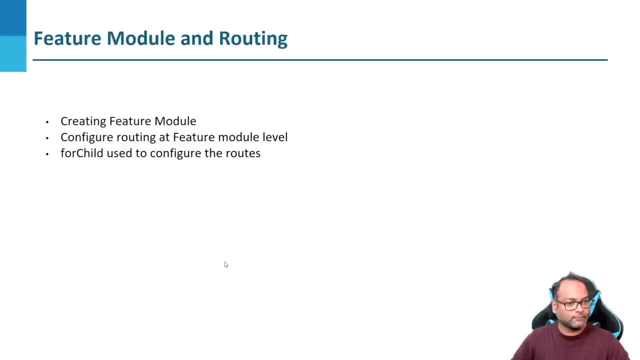 Just go ahead and redirect. So that's the difference. This is about router service. We will see more about router service soon, but not right now. In this video we are going to talk about feature module and routing, So remember so far what we have done. 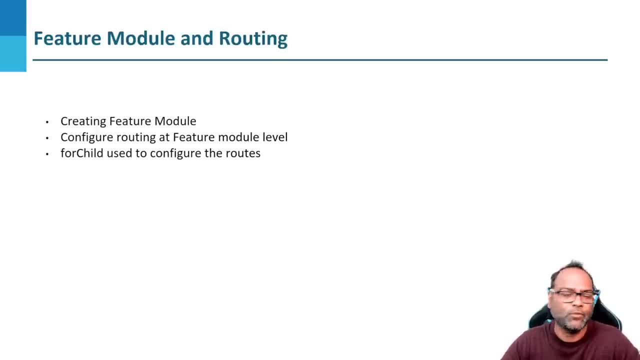 is we have single module, right. So we just have an app module which is available inside our code And that's it. But over the period of time the app module becomes like a huge code base that it really becomes difficult to manage it. 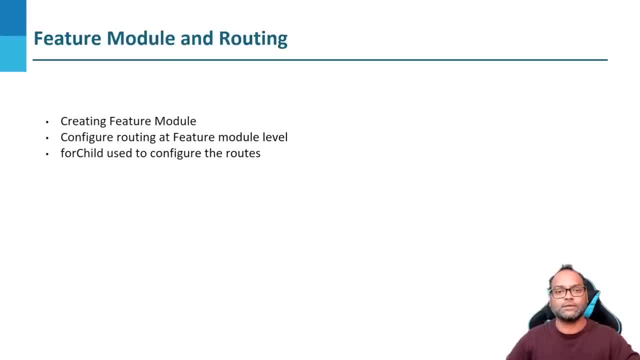 So that's where the concept of feature module comes in. So feature module, the concept of feature module, is you should actually wrap all the features together in a single module, for example if they are related. Sorry, I just missed that part. 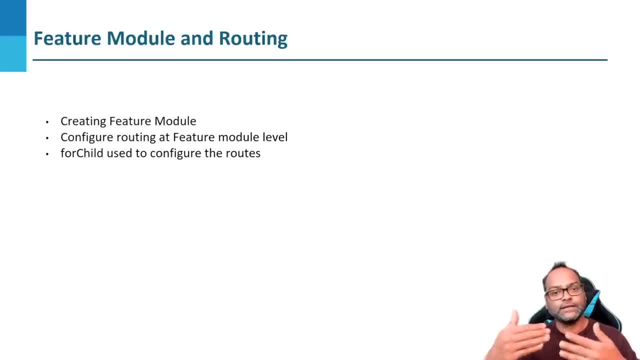 So if they are related- So, for example, rooms- So what I can do is I can create another module, move everything related to rooms inside that particular module, Sorry, Inside that particular module. The advantage of this is that it's not just a single module. 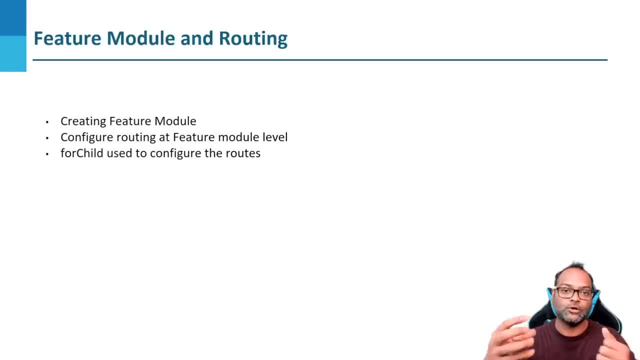 It's a single module. The advantage is, in case I want to use that particular module or some logic from that particular module, it becomes really easy to share those things. Also in future, in case we want to lazy load that particular module, which we'll talk about lazy load- 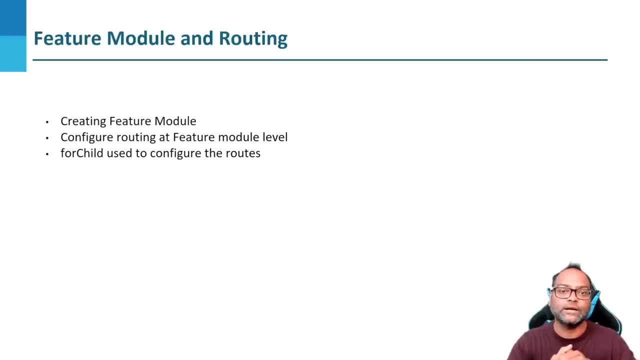 So don't worry about what lazy load is right now. But in case you want to do that, it really becomes easy to achieve lazy loading if you already have feature module. I always suggest, whenever you are working on some application, try to create your components and wrap it together using feature modules. 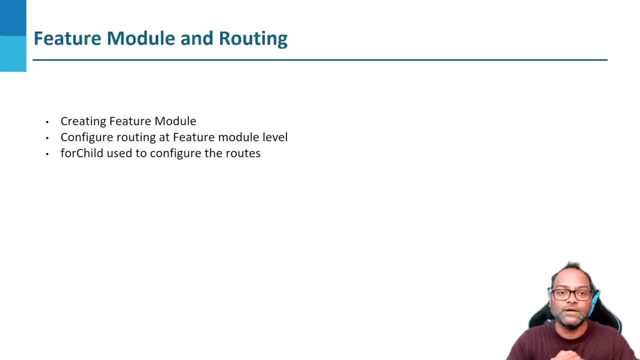 Or you can say modules. There is also a concept called SCAM, which is a single component and module which prefers that you should have: for every component you should have a module. That's also a very good thing to do, I mean in case you have a large application with thousands. 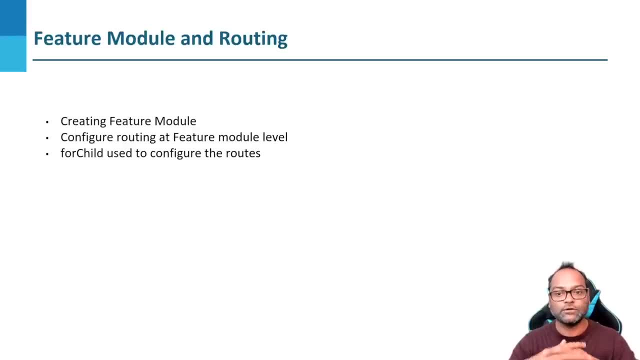 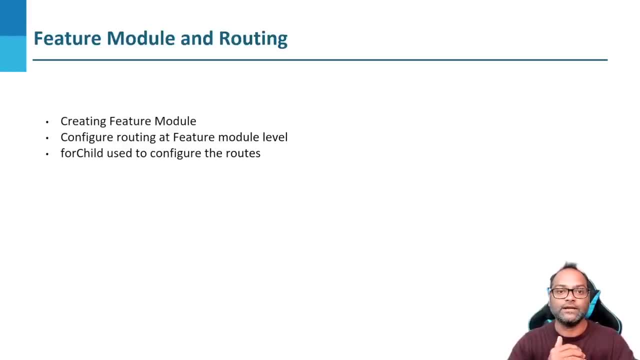 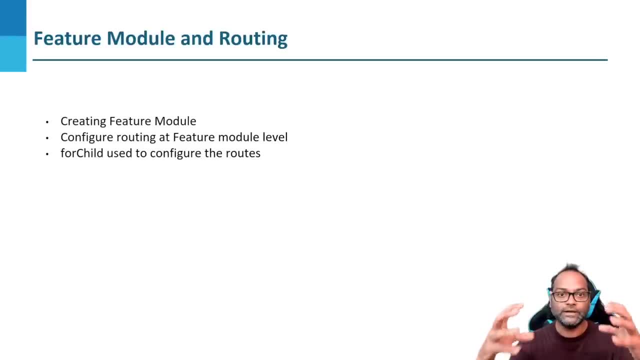 So always start with: think about: OK, if I'm creating this component where this component should fit in, Does it need a module, separate module? Just do that. In case it is already related to some feature, just go ahead and add that particular component. 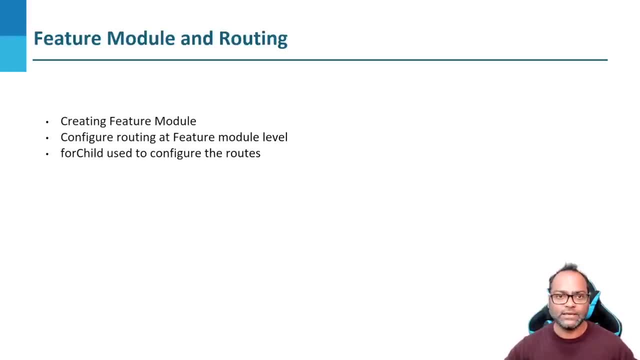 to that feature module. So let's start by actually breaking our rooms component because, remember, in most of the application, let's say, if you get assigned to any project, this may be a problem- that some feature is already created but everything is registered inside app module. so the first way i'm going to show you is how you will fix the scenario. 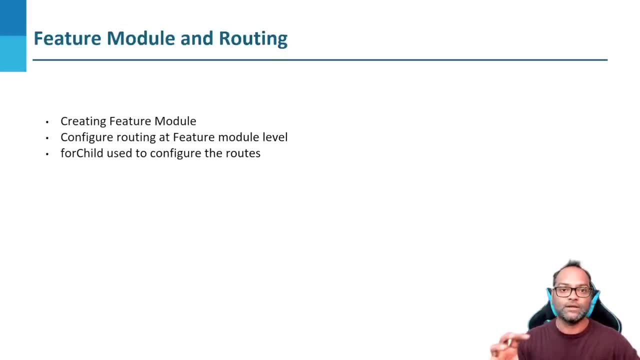 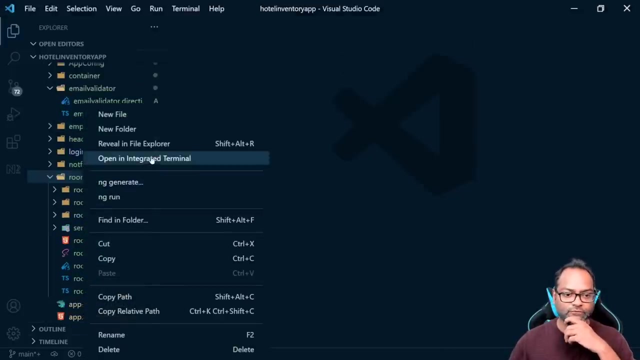 where you have some such concept right, where you have everything available into app module- for just example, our rooms. right now, everything related to rooms is actually registered into app module. we can actually remove that feature and create another module for rooms, right? so let's go ahead and start with that. so here we already have rooms folder. what i need to do is i need to. 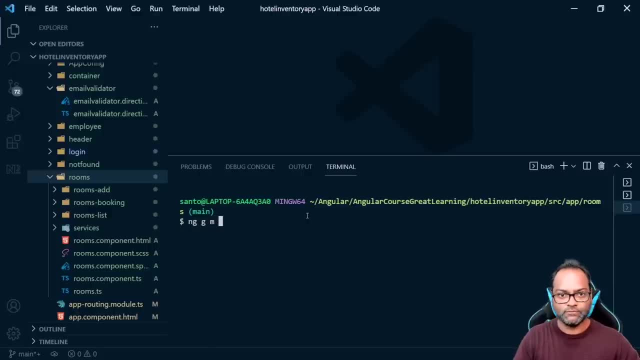 create a module. how you will create a module is ngg, m, m for module and then just give rooms and i will pass a flat equals to uh group. otherwise it will create a folder which we don't want to. we want that rooms module should be available here. 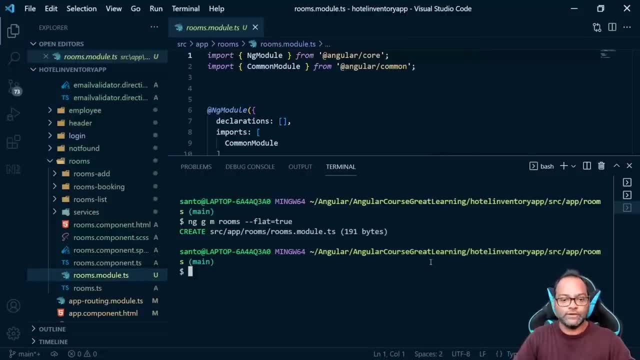 so we got our rooms module. uh, we want also wanted one more thing. we wanted, uh, that rooms should have a routing module as well, similar to what we have outside here- app routing module. so we want that rooms also should have a routing module. and we will say flat, true, and let's see. 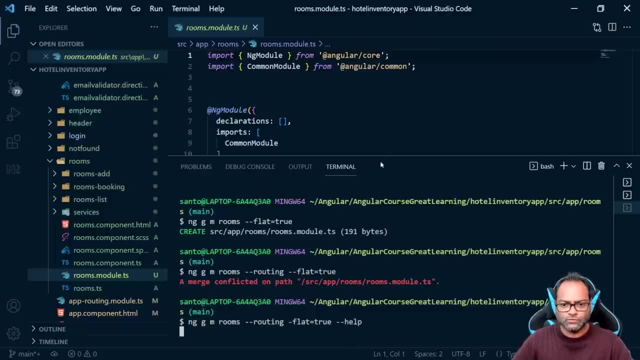 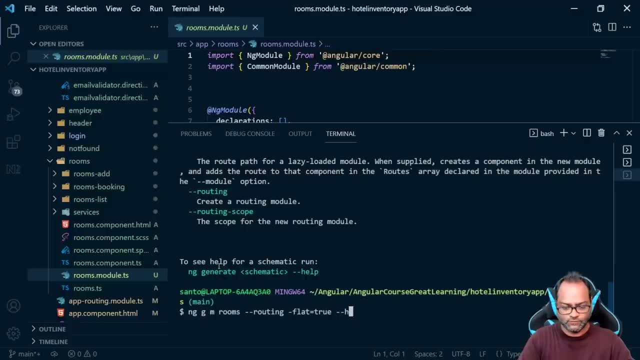 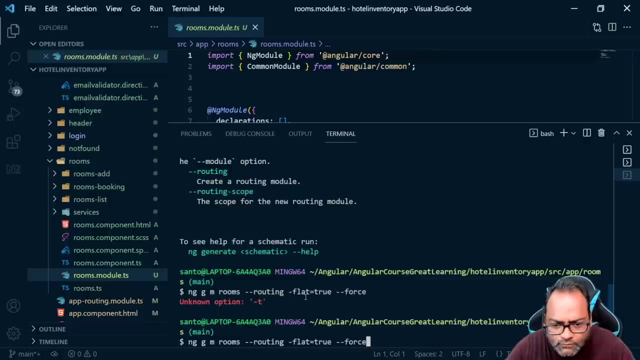 what it will achieve. so there is a flag to actually there is a flag to actually override. i'm just looking for that particular flag force. so i'll say, if force, so it will override the existing file. so we will have rooms module routing flat: true, unknown option. 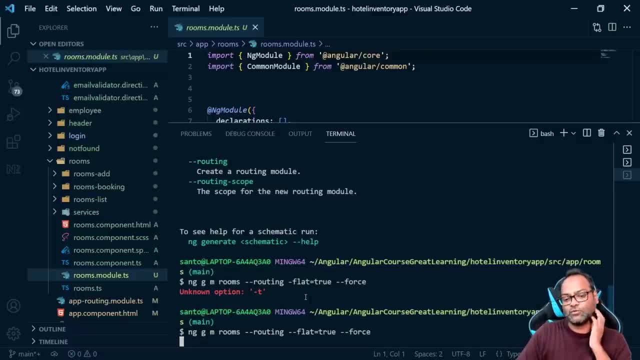 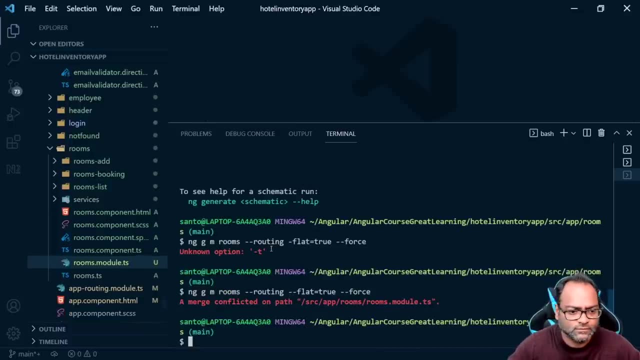 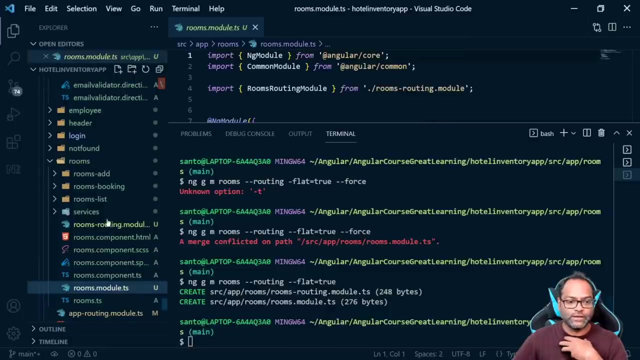 okay, sorry, because this is a i phone. i-phone flat equals to true, and then we have fn1 force merge conflicted rooms module. let's see? okay, let's delete this file right now. okay, so what we get is rooms module and room sorting module, similar to app module and apps. 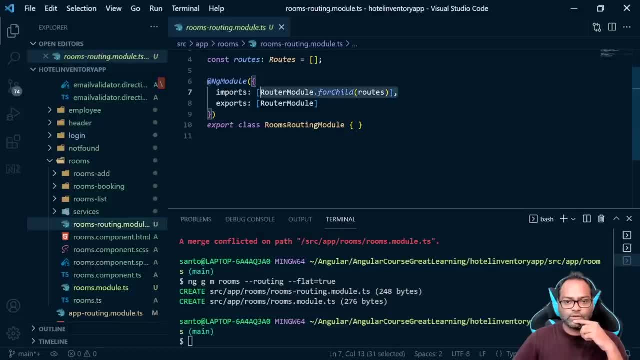 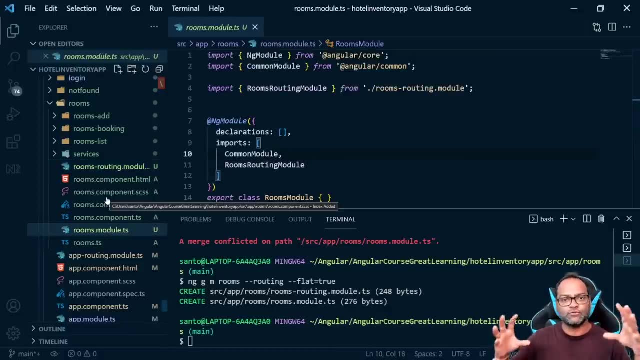 app routing module. but remember this: uh, we'll talk about this part for child. let's uh hold on. uh, first let's talk about this rooms module. now what we have to do is we have to move everything related to rooms out of app module to here. so let's go ahead and do that. 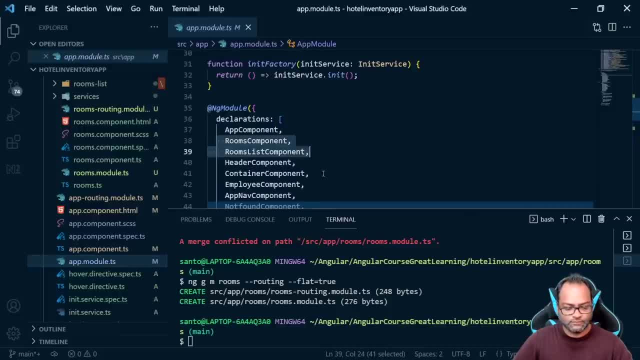 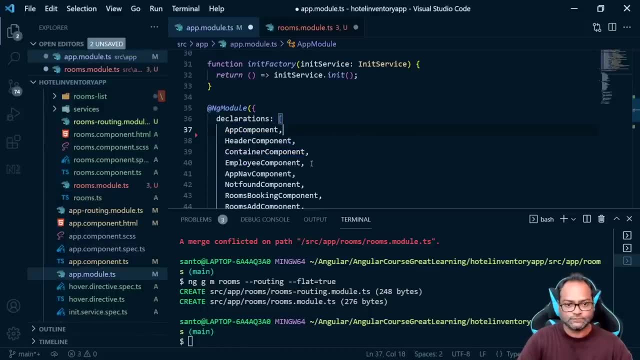 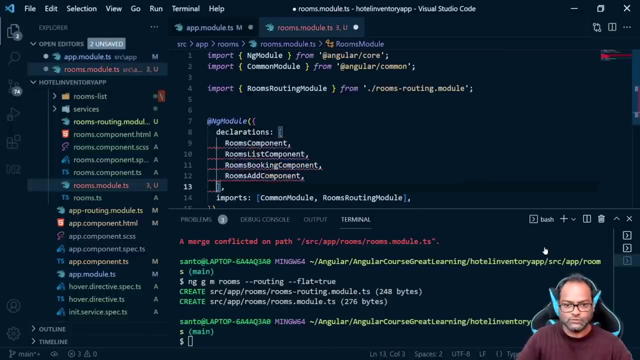 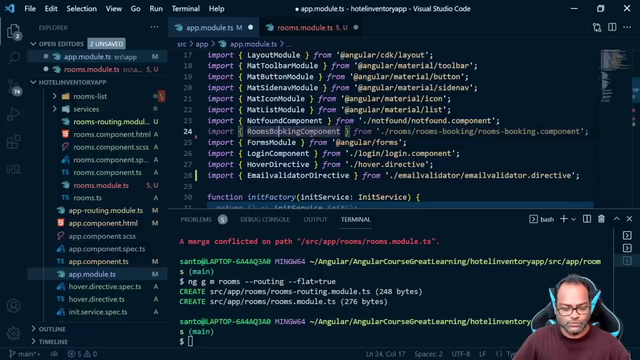 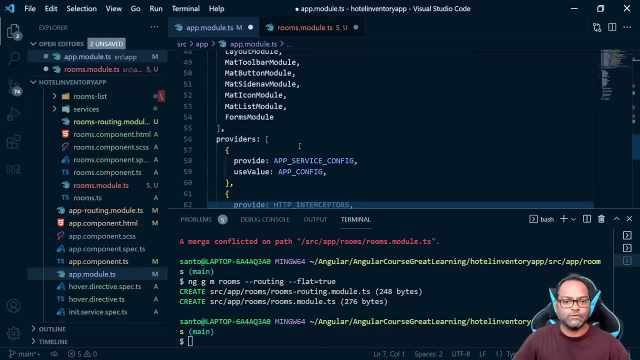 so we have rooms, rooms list component. let's do that. and what else? we have my employee rooms booking rooms ad. so let's go ahead and do that and let's remove this code. so you can see, just uh, by creating another component, i have removed like almost 10 lines of code from here, uh, from your app module. 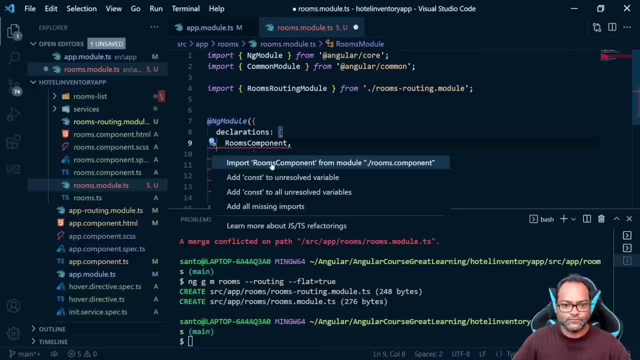 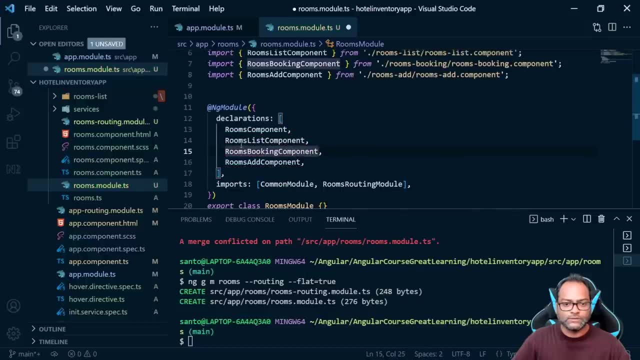 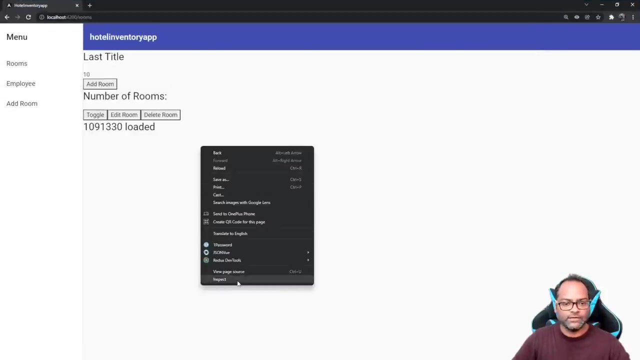 so now, this is step one. so now let's go ahead and add this, all this here, all these components are added here and we're going to add more of these. so what's going to happen is, uh, the application will break right now. so let's go ahead and see what is happening here and let's try to click on add room. 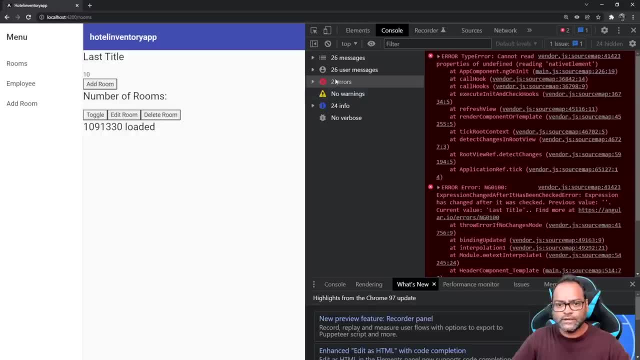 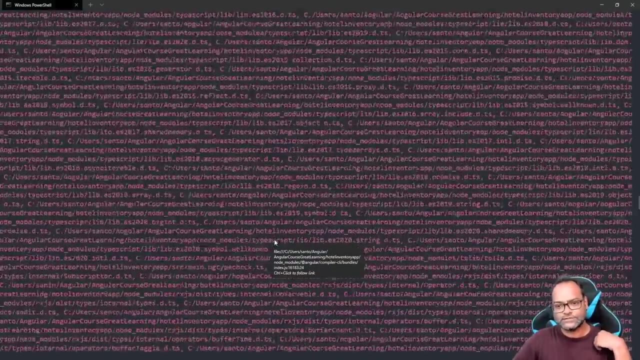 rooms. you can see nothing is getting loaded and you may get some exceptions, so native element, but it's okay. but you can see, i mean there's nothing which is getting loaded because, of course, uh, there is a lot of errors, a lot of compilation errors, so let's go ahead and try to fix those. i 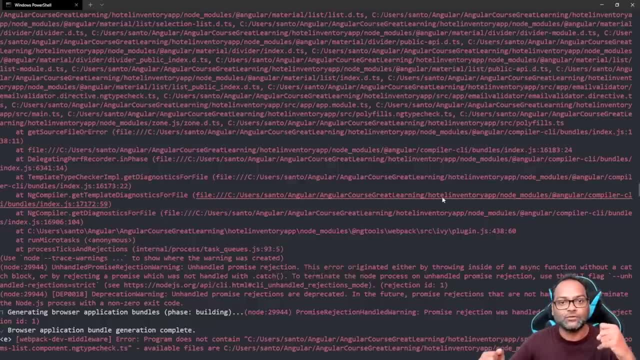 about refactoring. I'm also trying to show you how to refactor the code base. You are probably- I mean, it's a good thing, You should always revisit your code base. So I'm just trying to tell you how you generally- I generally- go ahead and refactor the code base. So now we have a lot. 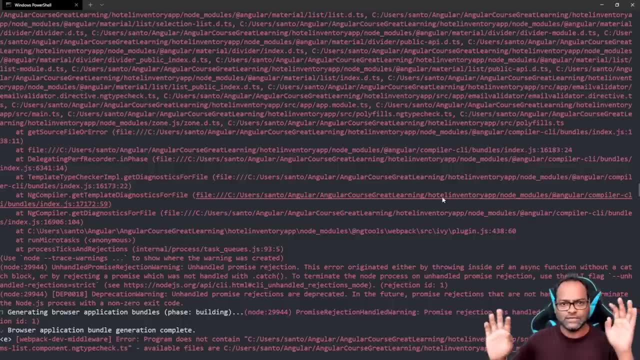 of errors. Don't be scared. Whenever you see such errors, don't be scared. I mean it's absolutely fine. That's the first step. If you are scared, I mean of course you will end up like you will. 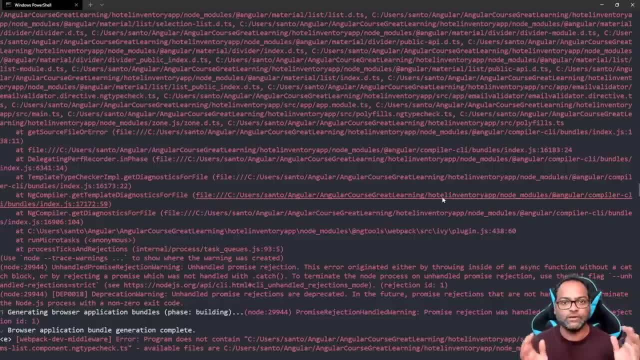 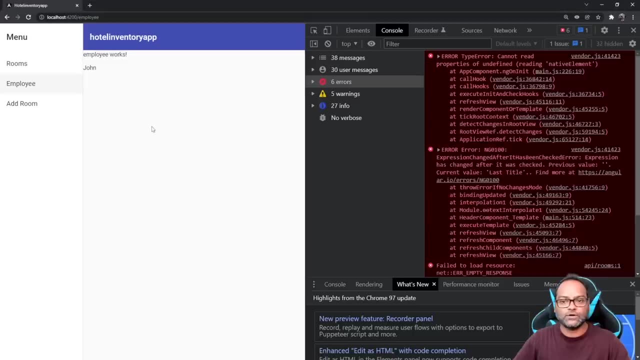 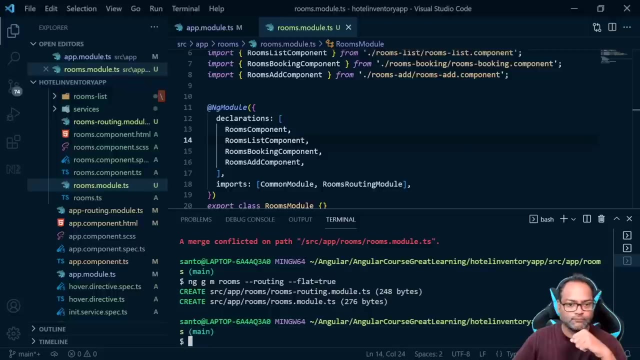 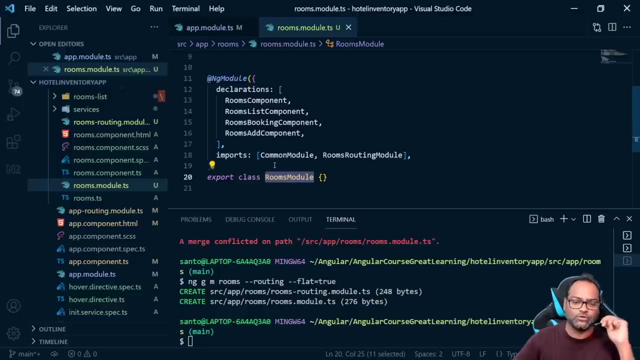 roll back the code base and you will be in the same mess as you were earlier. So now let's close this and let's try to see what needs to be done more. So we have moved all the components here now. So we have all the components here And now, as we have created just a feature module. 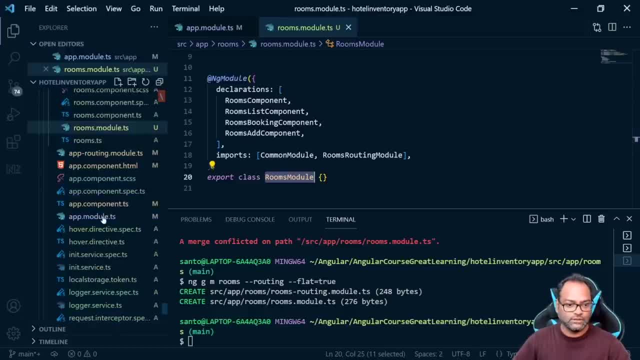 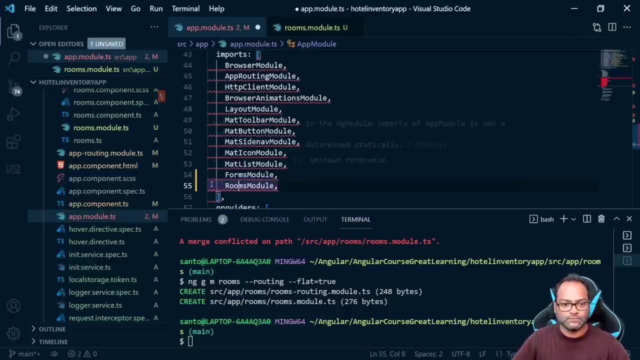 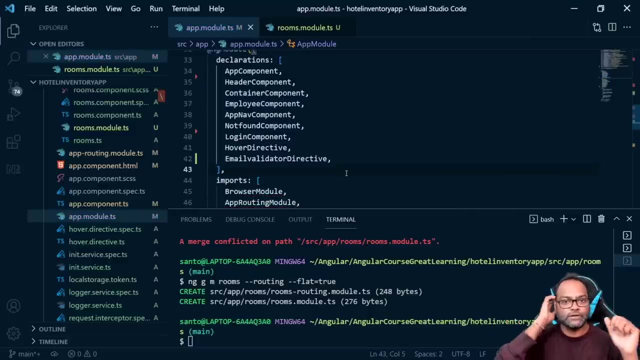 what we can do is we can actually go ahead and register this rooms module into this app module. So what we have done is we have removed some code from your app module and then we created another module And as we want that module to be available everywhere, 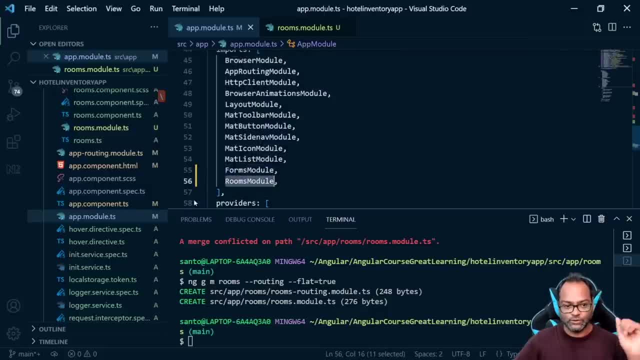 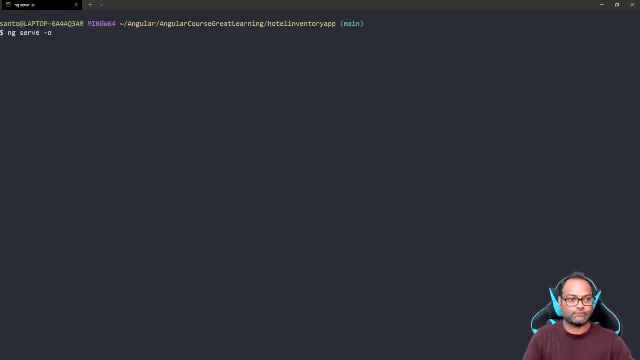 we have just registered that module here, rooms module. So let's go ahead and compile this code again. So what you can do is you can actually put some of your reusable code inside a module And then you can just use that module wherever you want to, In case, let's say, you have a component to 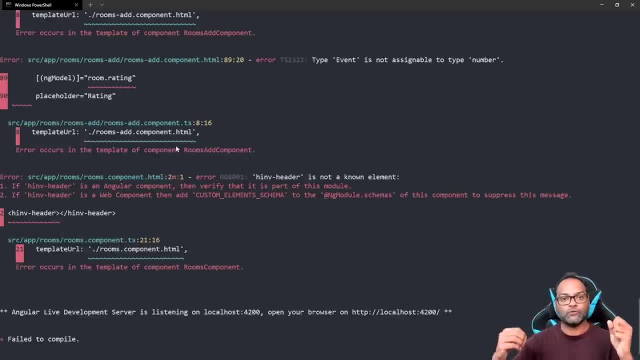 show a table And what you can do is that table is getting used at many places. So what you can do is you can just create that particular component with table and a module And then you can just use that module everywhere where you want to. 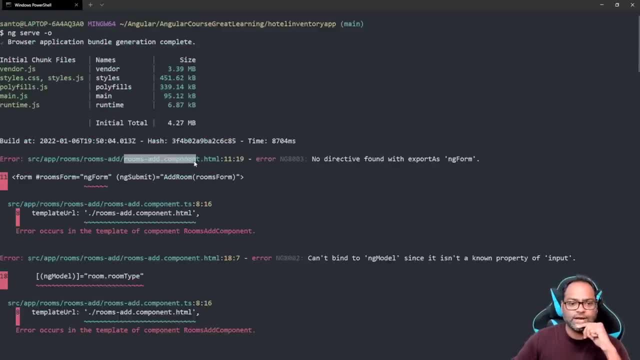 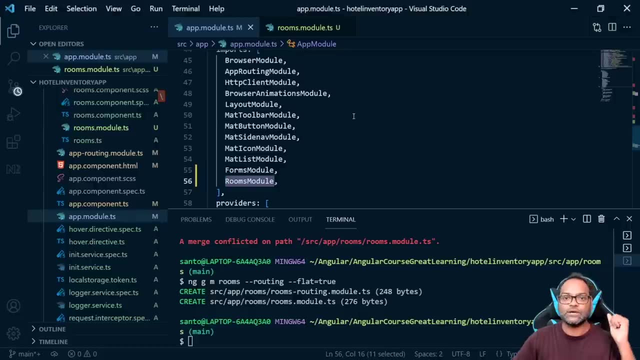 So let's go ahead and see the errors. So there are multiple errors. So it says rooms add component: no directive found for ng form. Now, once you create a module, there are few things which you have, to which there are a few things which you have to keep in your mind. Now, this components: 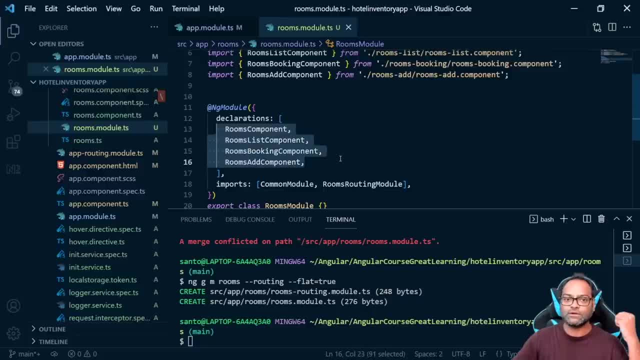 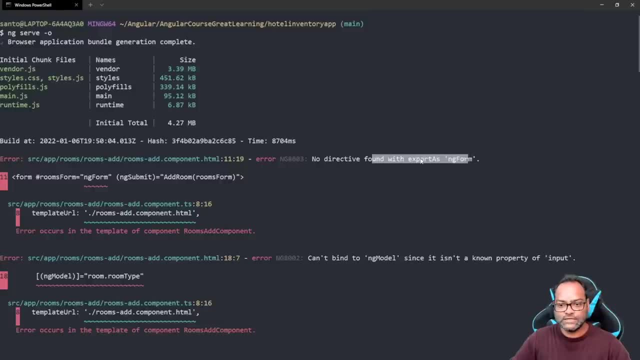 which are available here. they are using some specific modules, For example, this error. this error which says: okay, there's no directive found with export as ng form. It means we are using form functionality here, but that form functionality is not available. 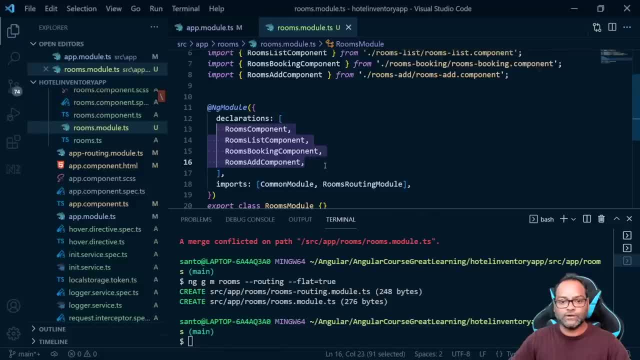 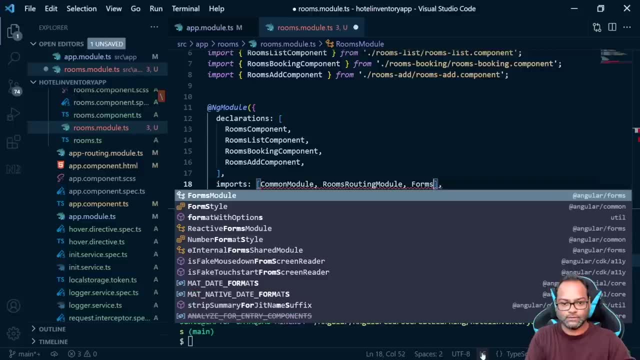 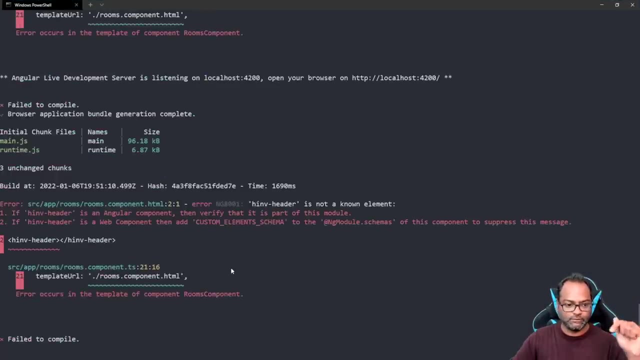 How you can do that. We have already learned about it. So what we have to do is we have to go ahead and add into imports- We have to say forms module, So you will see each error gone one by one. So now the first error will be gone, So it will be recompiled. failed to recompile. 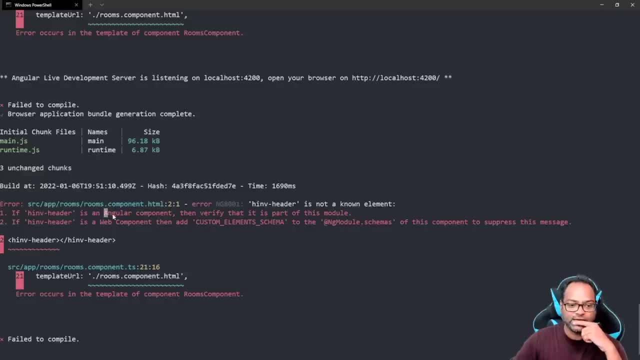 And now there is another error. It says this header component is not part of this module. Now we are using this header component in rooms componenthtml. This is a really good use case for a reusable module As rooms component. sorry, this header component can be used at multiple. 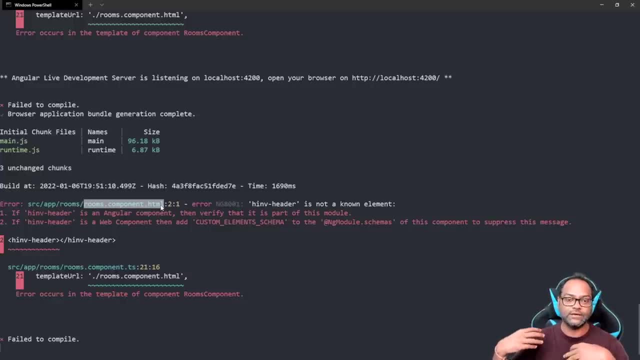 places. We cannot just register it inside the main module, app module- Otherwise it won't be available for other modules which is created, for example, rooms. So what we can do is, in such cases, the same example which I was giving: our table: a reusable table, which is a reusable table. 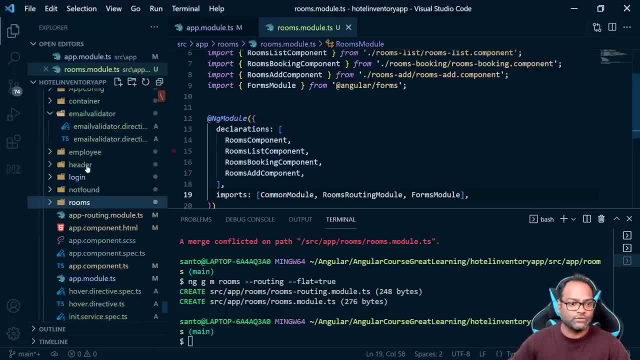 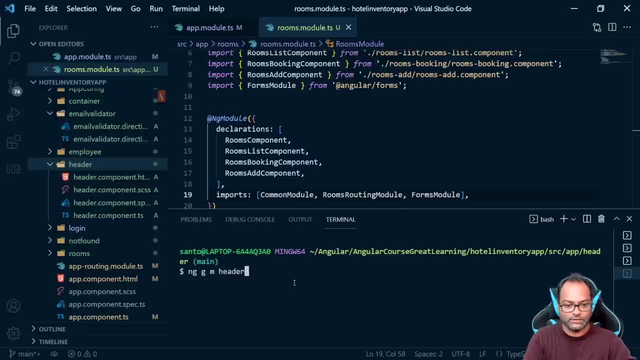 which can be used. So here, uh, what I can do is I can just go to header. I can say: open an integrated terminal and create a module here. So I'll say this is a header. I can, I can black. 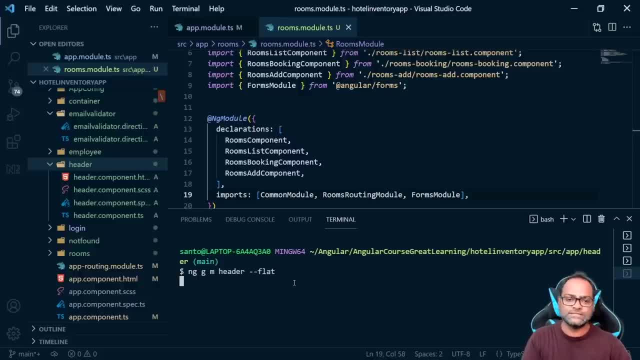 but I don't need a routing module here, because this is a just a usable component. It does not contain any component which can be accessed by route. The reason I created inside room is there are components which can be accessed by route, by URLs, So we will also move the. 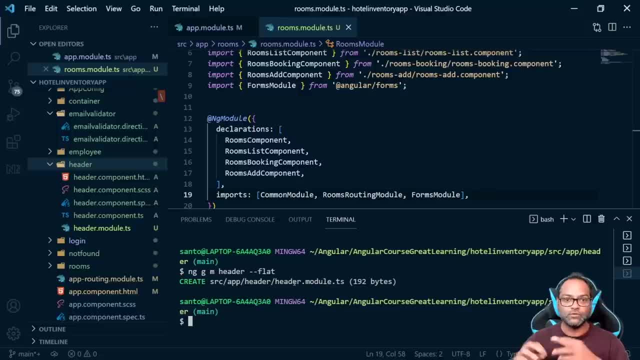 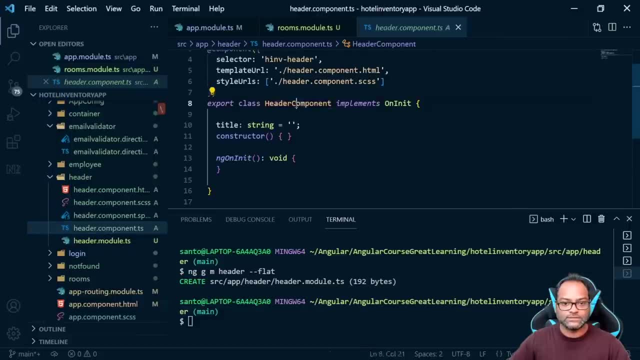 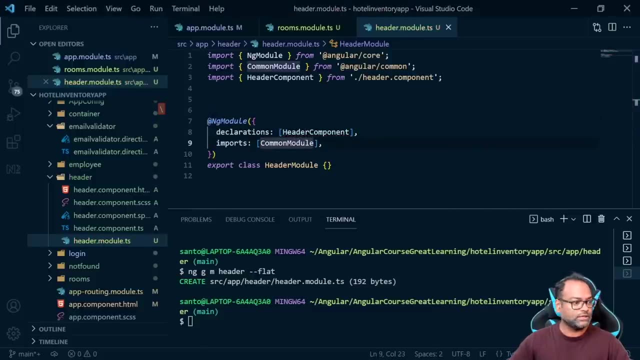 logic related to the URLs inside its own module, to avoid writing so much code inside your, inside your app module. Now, let's register this header component here Now. once you do this, you will start getting in effort. So the thing is, one component can be. 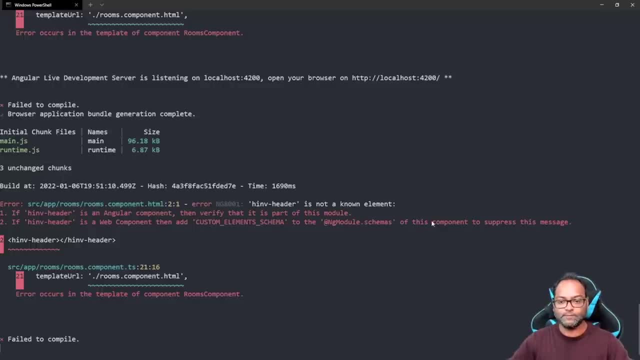 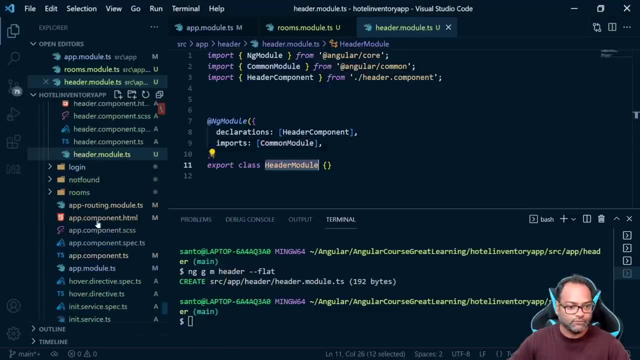 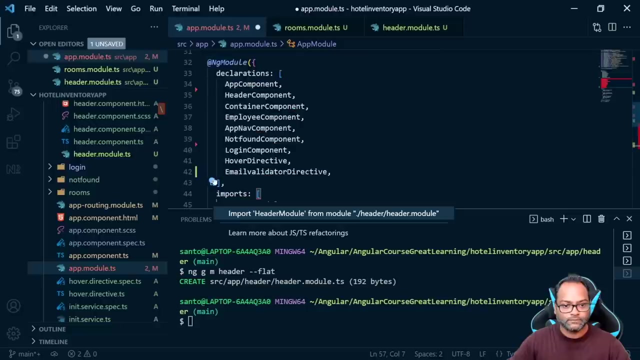 registered as part of only one module. Remember this, keep in your mind. So here, uh, the center component is actually: uh, if I, if I do this, So if I do here, I register the setter module and let's add the setter module here. 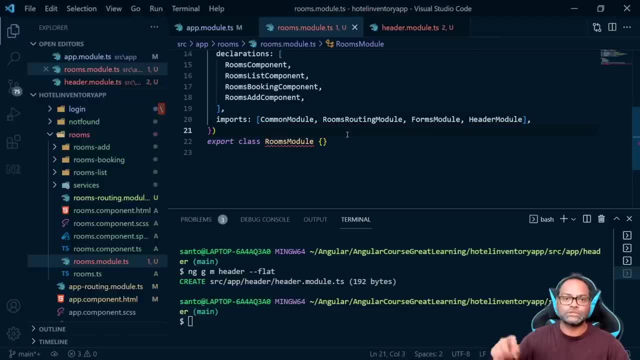 So the thing is your imports or your modules can be added into multiple places. right, And that's the whole. you can say that's the whole core about creating the module, So you can actually reuse things around your entire application into multiple modules. 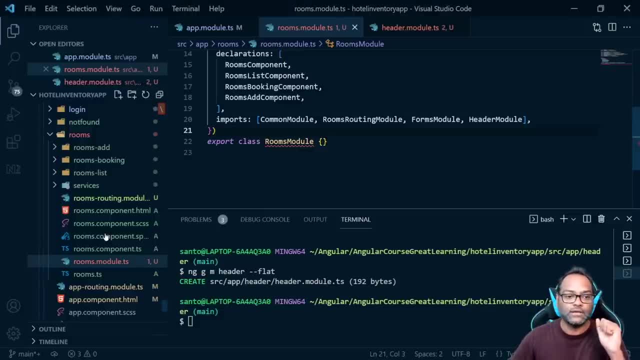 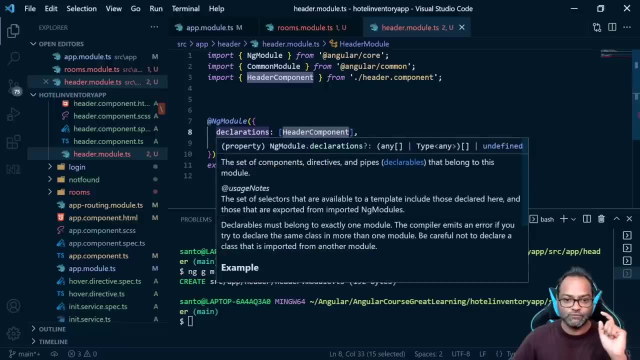 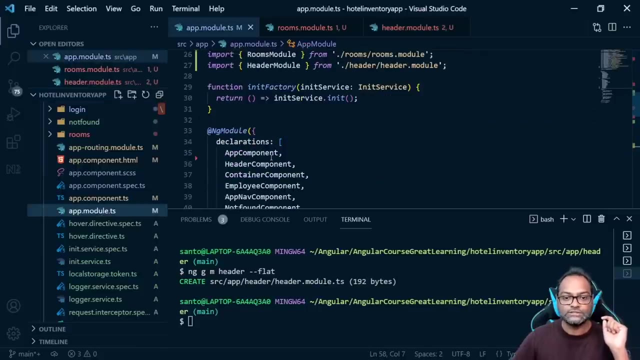 But I cannot register or I cannot actually import. sorry, I cannot register a component multiple times. So if I have added declarations header component into declarations array here, I cannot add it into here. So If I do this, that's an error. 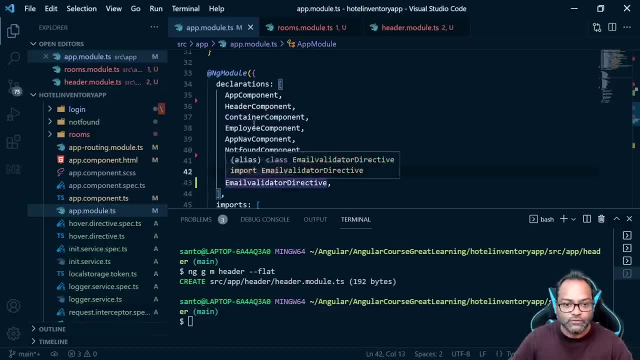 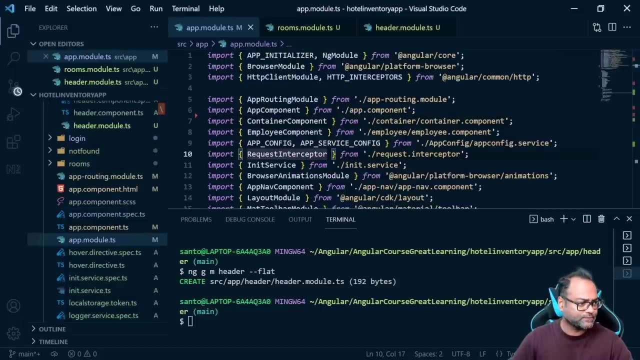 So here let's remove this over header component from here, right? So header component is removed And now it's only available at one place. But let's see if it fixes our issues, So I'll just compile it again. 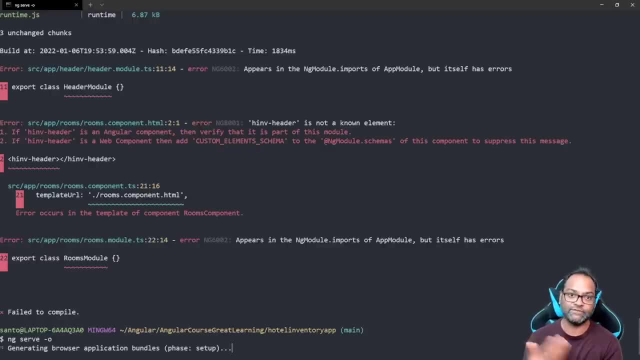 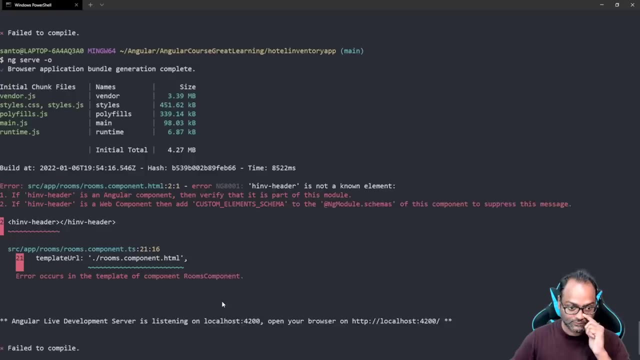 It will not. So the answer is: it will not, So we'll see how we can fix that. So now let's let it give us the error first, So let's see how we can fix that. So let's see how we can fix that. 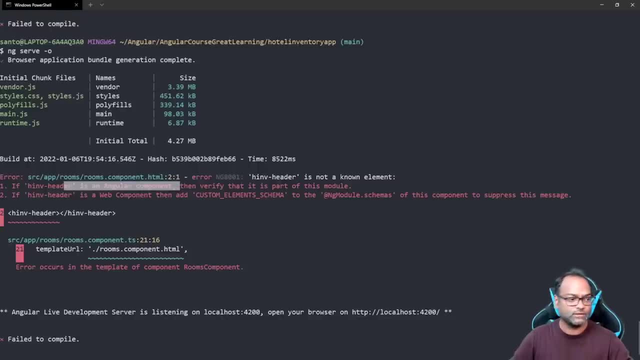 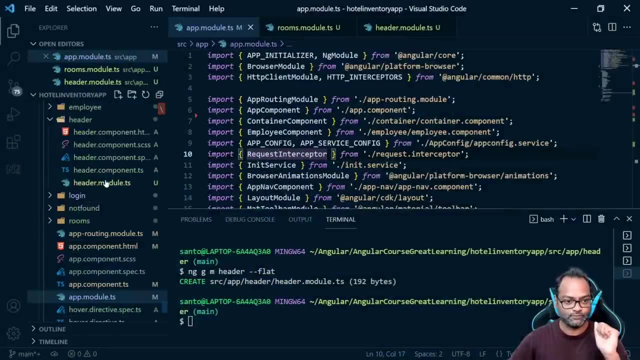 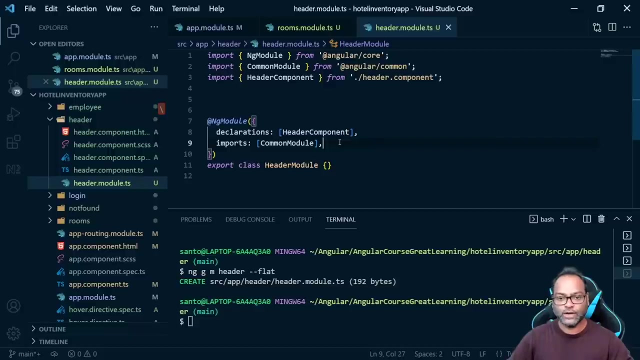 Now it says: okay, this header is still not found, The reason being in case, if you are using a component outside of its module, So this header component is actually used inside rooms module, So you have to also add it to exports. 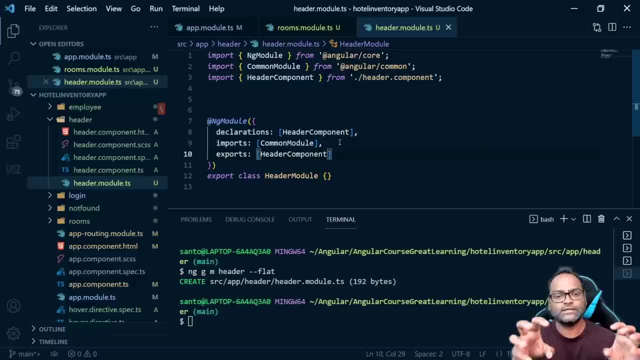 It means I'm exporting this particular component, So anyone outside this module can also access to this, This particular element. Remember this: Whenever you are creating reusable components, this is the thing which you should do. You should always add it to exports array. 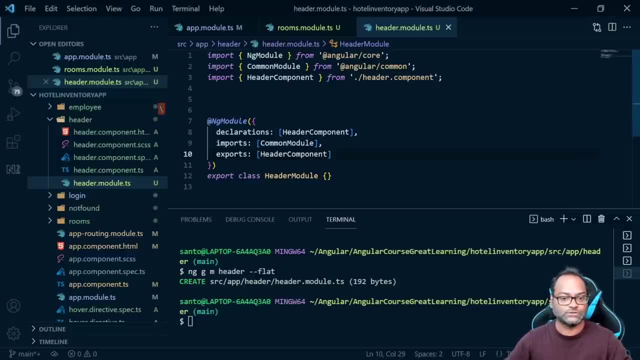 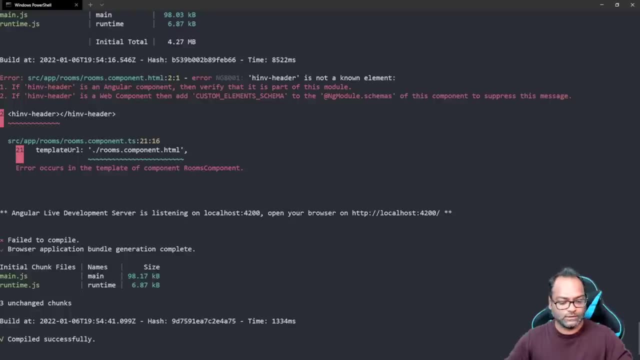 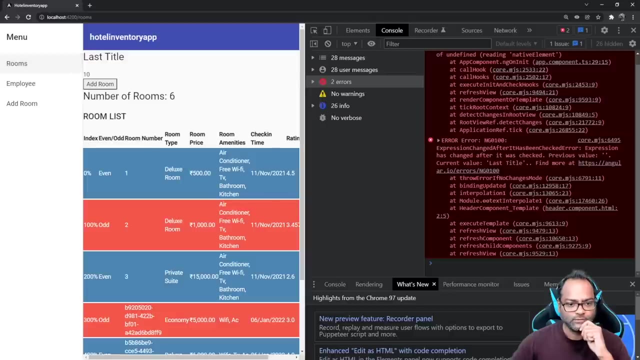 So it can be accessed outside. Otherwise it won't be available. Now let's go ahead and see our output. And it is compiled successfully. So let's see if our application works. Rooms Worked- Add rooms. 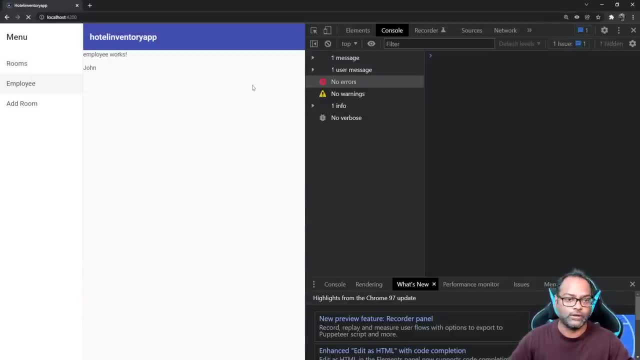 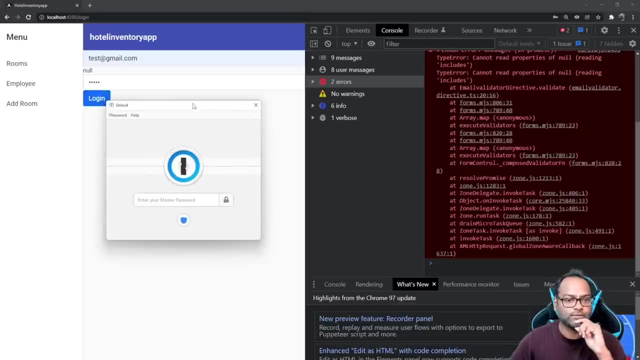 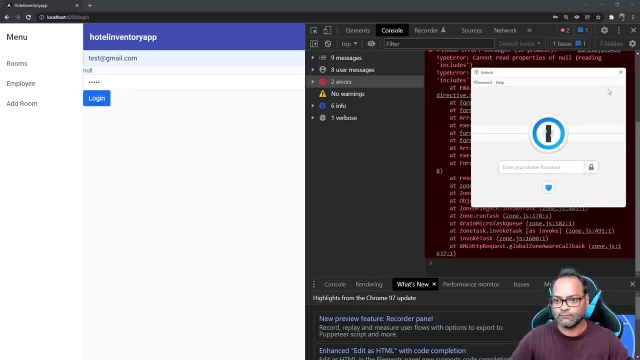 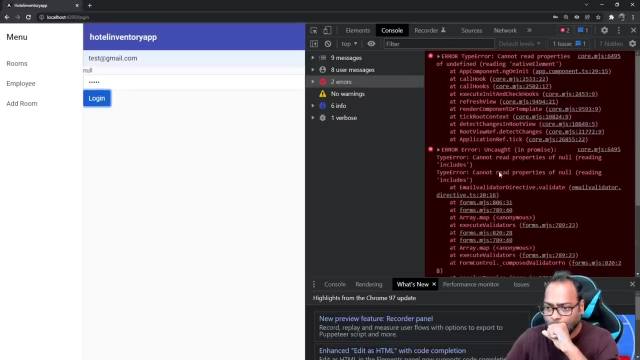 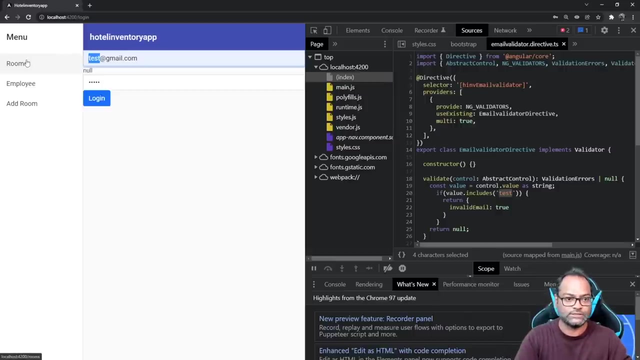 Worked. Employee Worked. Login Worked. Let's try the functionality. Okay, Looks like something is broken, but okay, It says includes test. This is right, So it is given. So it is giving us error. 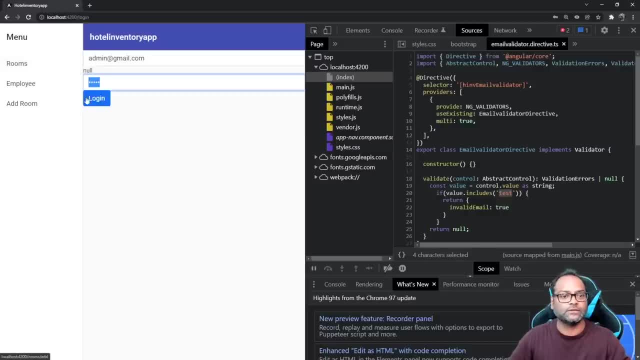 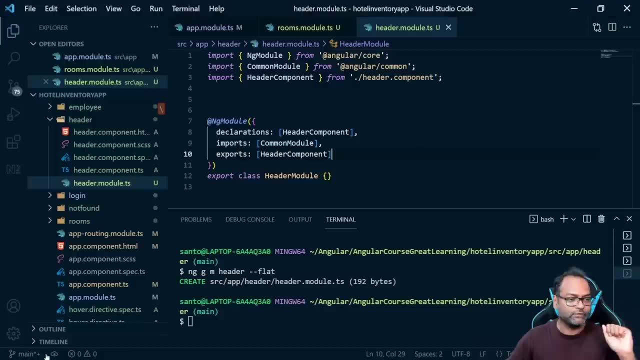 What was the admin? It was admin right, And now it works as well. So entire functionality is working again. What we have done here is we have created actually two feature modules: One to show the scenario where we will not have any routing module. 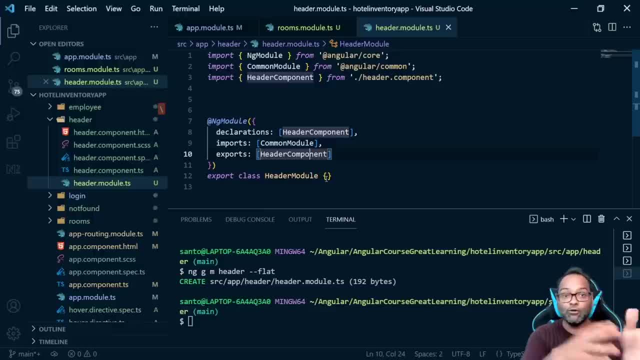 We will have a component which is reusable and can be accessed outside of its own module, So it's not going to be used inside its own module here, right Header module. And then we saw that it's not going to be used inside its own module. 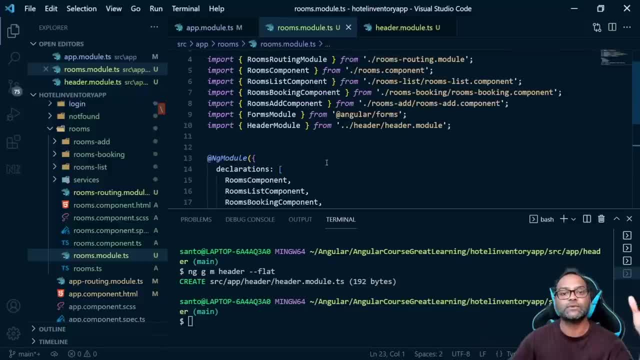 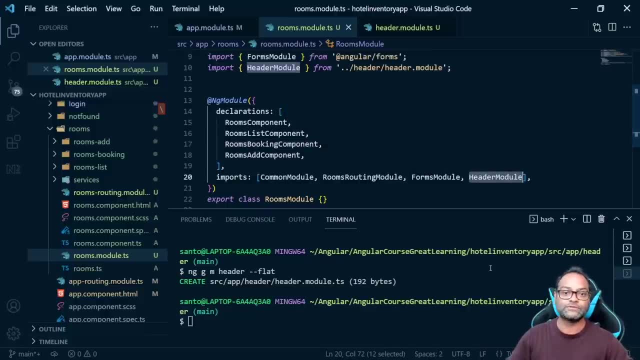 So we saw another example where we created a rooms module. We moved all the components which is related to rooms module inside its own module And that's it. And then we also added the modules which is required here. For example, it was using the forms functionality. 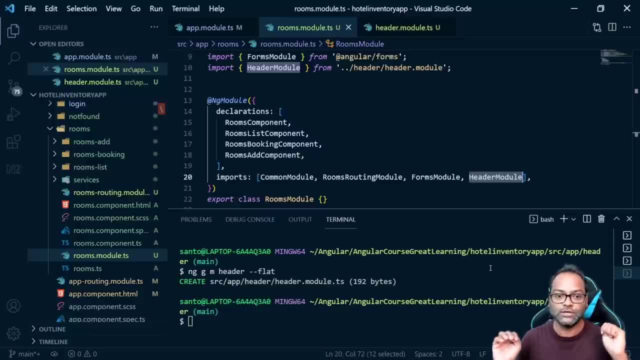 It was using the header component, So we added both the modules to make it successful. Always read the error. Remember, whenever you are effecting the code, always read the errors. What is that? All the errors are readable, So you know what is going wrong. 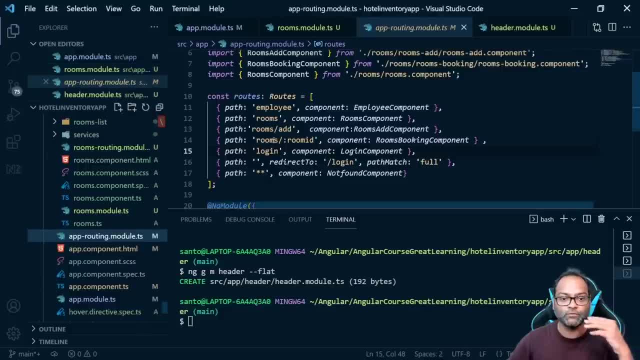 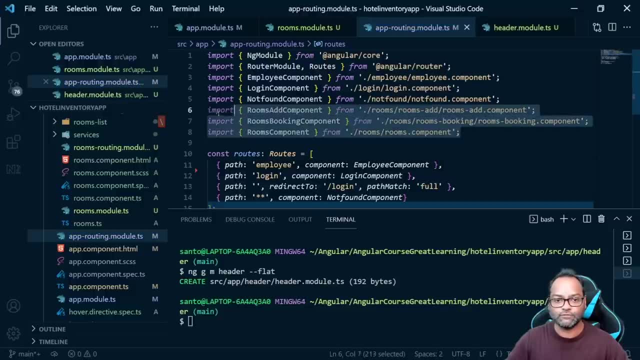 Now let's move ahead and also try to move this rooms-related routes to its own module. So we already have this module available. We'll remove it from here. So you can see how easily we are able to remove a lot of code from our app module and app routing module. 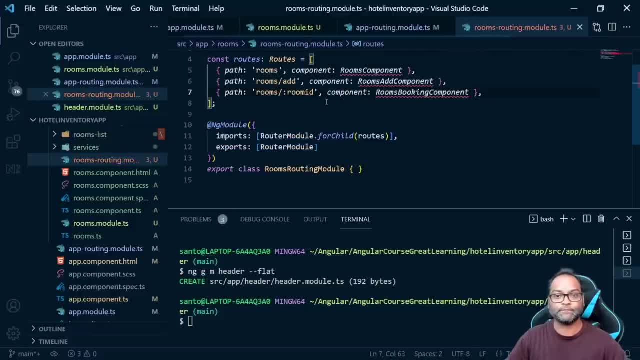 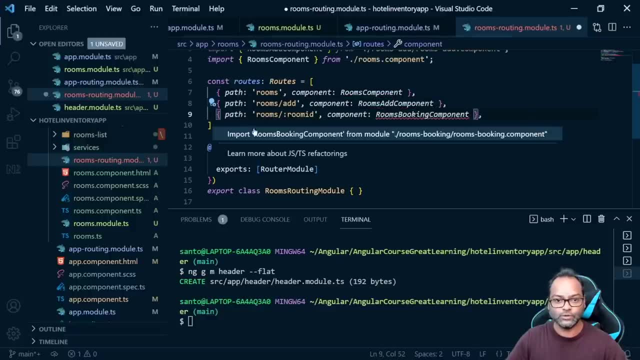 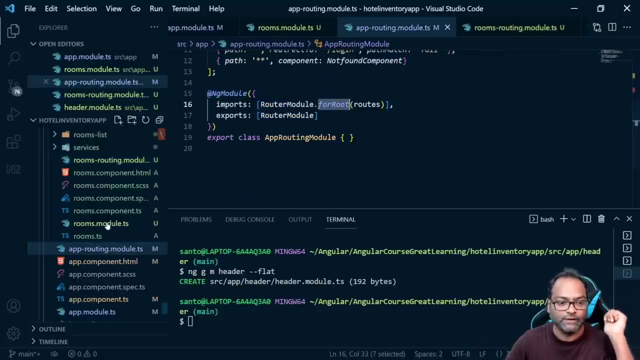 And we will add it here. So rooms, component rooms: add component and booking component. Once done, you will see a difference that in app routing module we always use for route And whenever you have a feature module with routing, it will always use for feature. 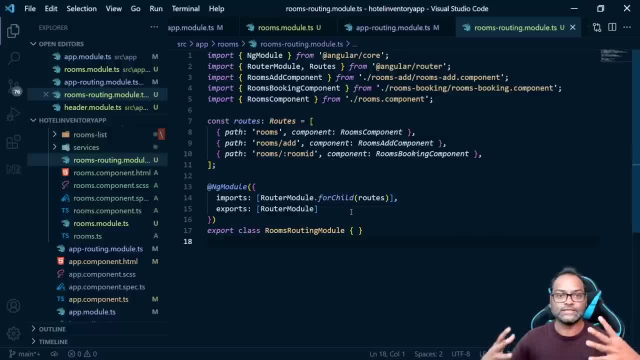 Sorry for check. The reason being your for route is like it's a singleton service, So you are adding all the routes inside a singleton service. So we are saying for route It means these are the routes which are available globally. 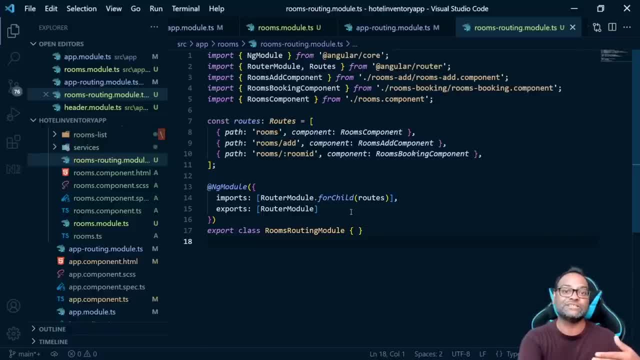 And all other routes is part of your feature modules. They can be accessed from within your feature Or, once they are routed, they can be added to your feature module, So once they are registered. so here we have three routes which are available and the way it works is routing module is actually registered here. 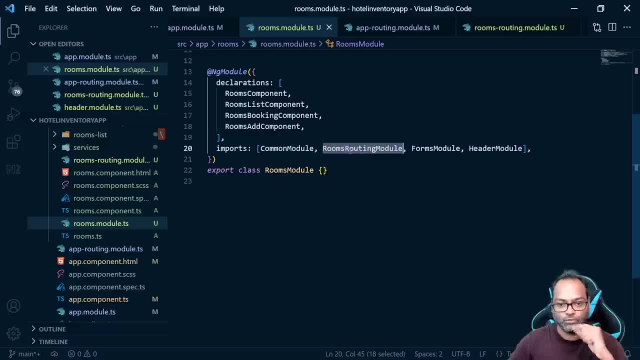 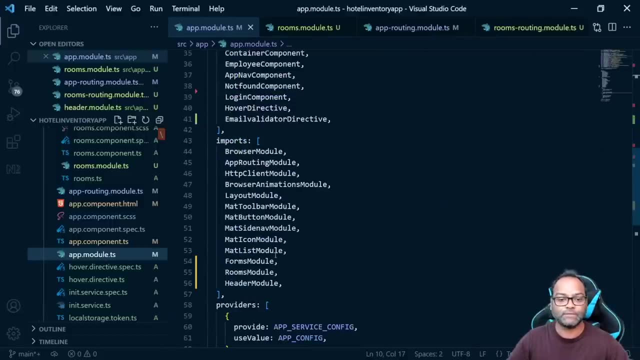 You can see imports and we have added a rooms routing module, So now this routes are also registered. but there is a catch. There is a catch, Let's see. We have added rooms module here. Let's go ahead and see if our application works. 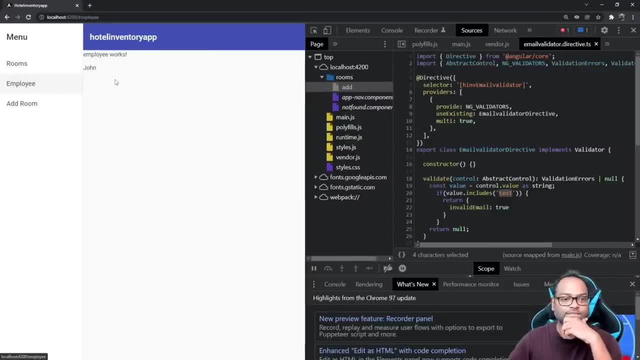 It will break. So just to give you an idea, So you can see: if I try to access employee, it works. If I try to access rooms, it says resource you are looking for does not exist. Same for add room. 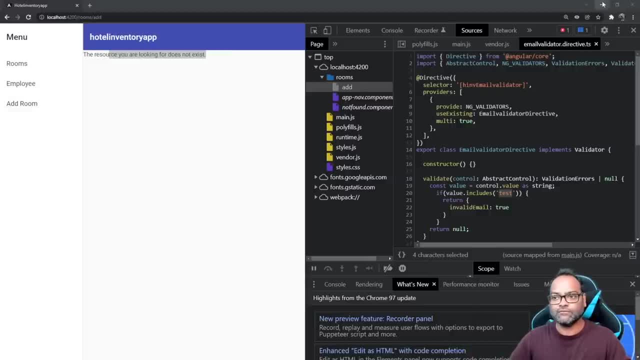 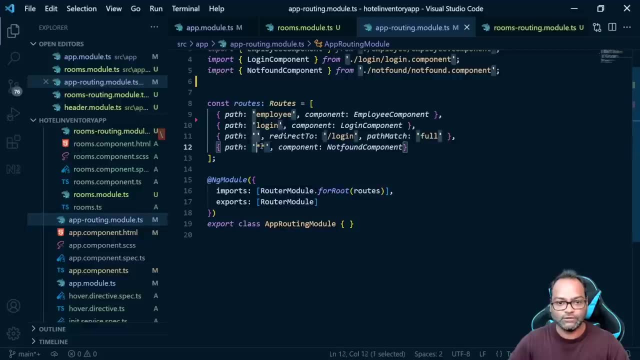 What's happening here? The routes exist, yes, but why we are getting 404?? Let's go back revisit the basics. Remember, when we were talking about this routing right, We talked about this wildcard. We said it will go sequentially from top to bottom. 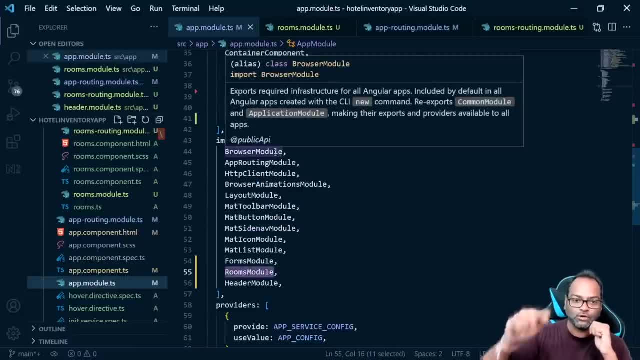 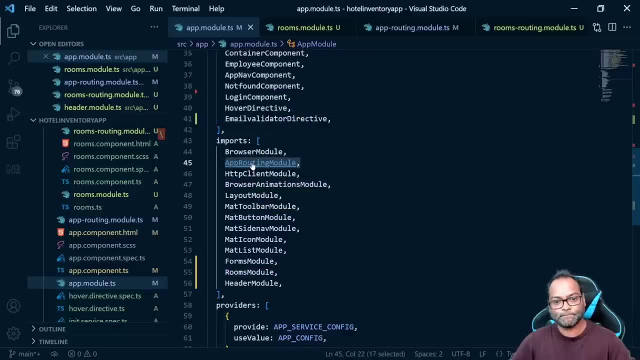 Let's go to app module and try to figure out why it is happening. So all the import statements are also executed sequentially. So you can see It goes to app routing module first and goes to app routing module. it says okay, employee login this default route and then start. 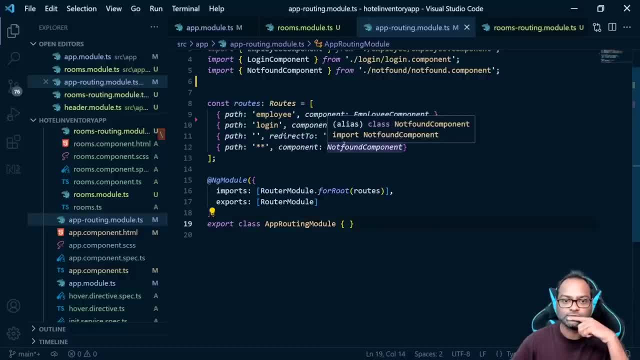 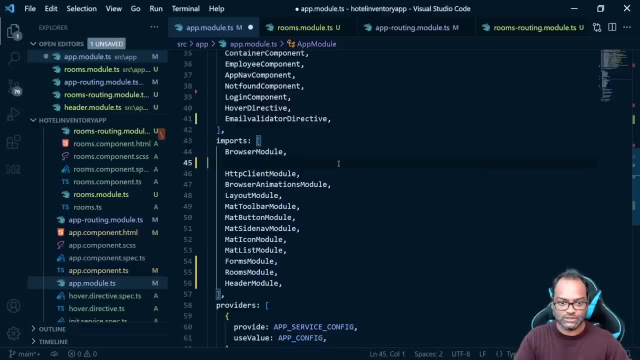 It says okay, the. any other route is not available here right now. So how to fix it? So, in case you have feature modules with its own routing, you should always register this. You should always register your feature modules before app routing module. 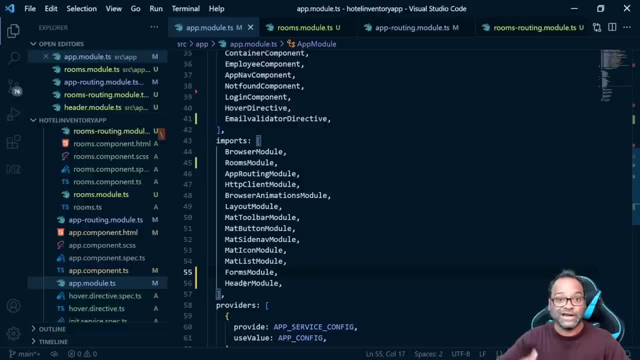 Just remember this, Because, of course, When you start learning Angular, you will get this error. you will get: okay, why my routes are not working, that this is. this might be one of the reason that you are getting 404 pages. 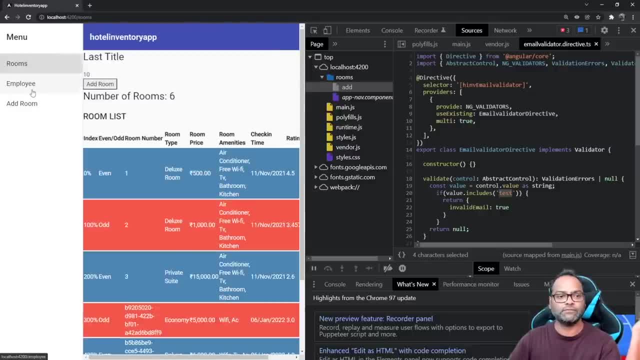 Let's go back and that's it. Everything back to normal And your functionality works. So this is how you can create a feature module, and and also how you can create a feature module with its own routing module. So remember right now what we did is right now what we did. we just did is we refactored a code. 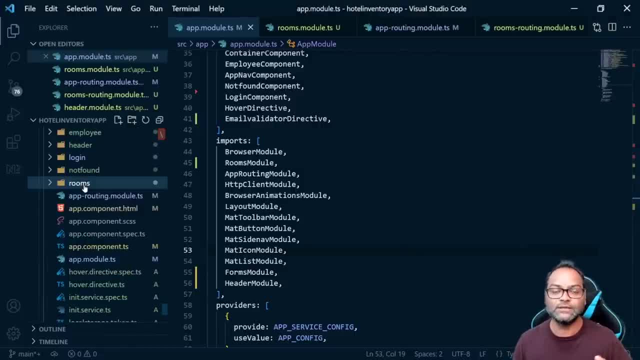 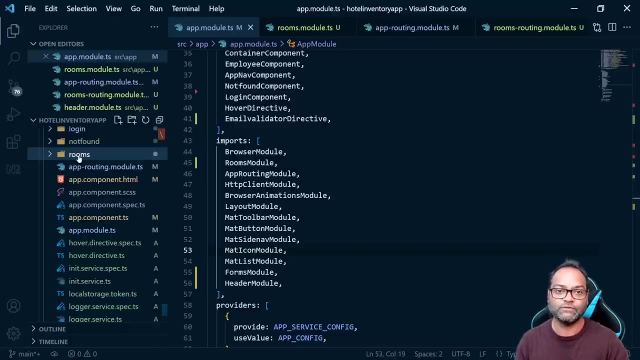 Base to make it more- what you can say- flexible, more extensive, extensible. So in case anyone wants to actually make changes to related rooms, they know that they have to just make changes inside this particular folder. That's the whole idea about creating this small, small feature module thread. 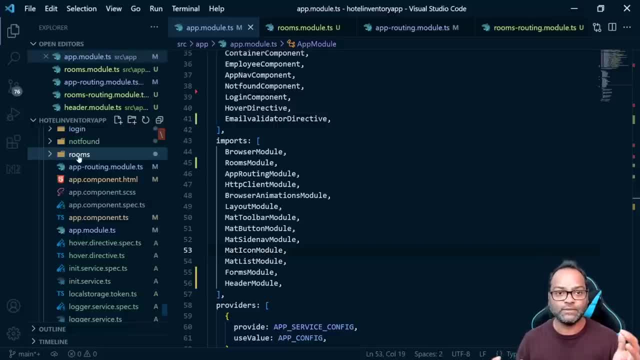 People know where to make the changes. They don't have to touch the entire application. They don't have to make changes into app module every time. That's a really bad structure in case you get into some code base where everything is added into app. 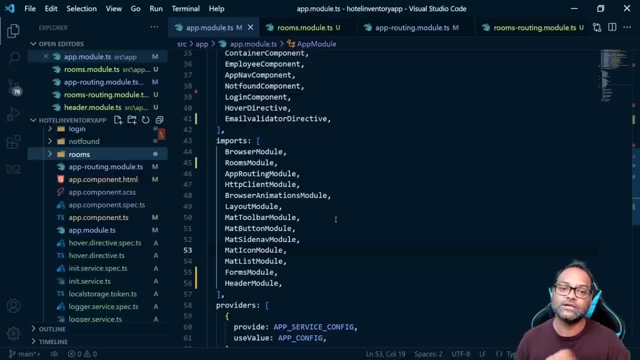 Module? Of course you should. the first thing which you should suggest is to refactor that code base by splitting them into different feature modules. The advantage is, of course, the code is more maintainable and we can also do lazy loading, which we will see later on. 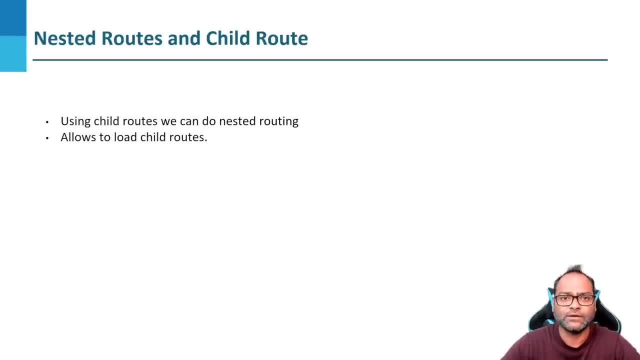 Now in this video we will see how we can do nested routes and we can load child routes. So let's see, let's try to understand what we mean by nested routes, right, So we can Load another route inside an existing route. that's nested routes and it can have some child routes as well. 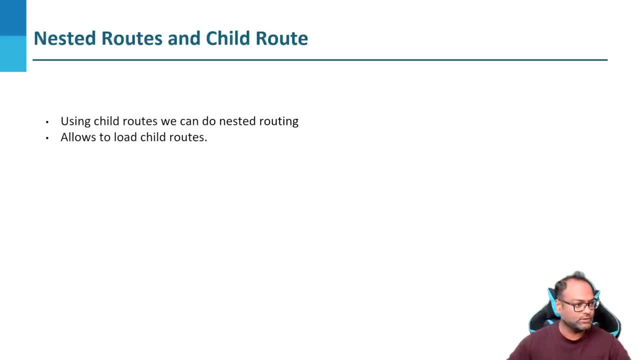 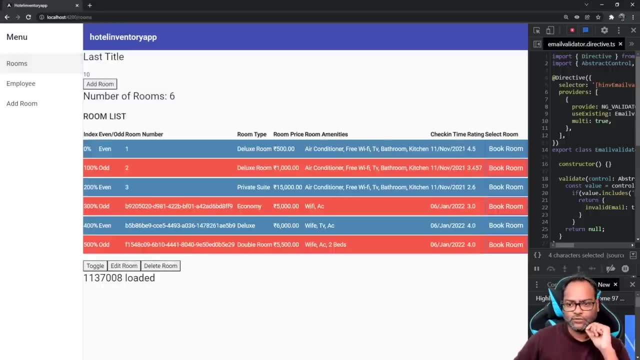 So let's go ahead and try to figure out a scenario. So here, So you have this book room, right, right? So right now, if I click on this book room, it is going to another view altogether, right? 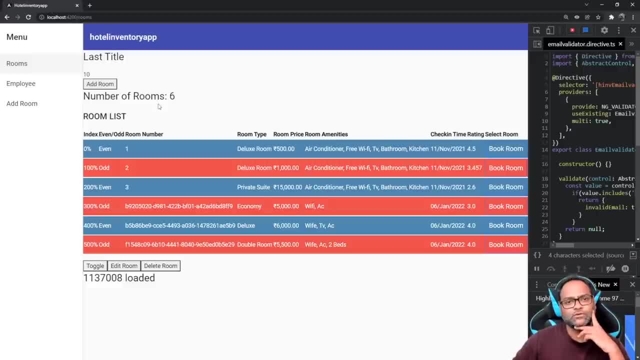 So all the existing view is lost. So what in case you get a requirement that? what in case you get a requirement that when you, When you click on this book room, the another view should open below this particular table, so you can just fill out all the details and complete the booking? 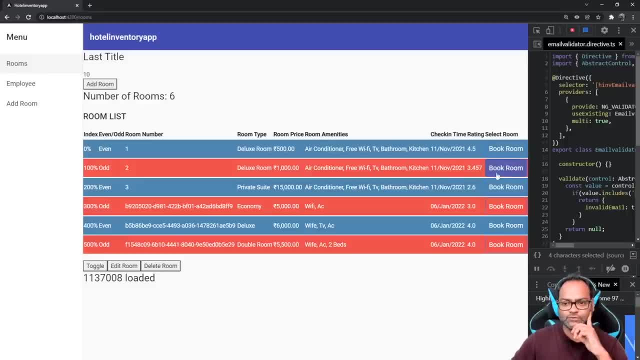 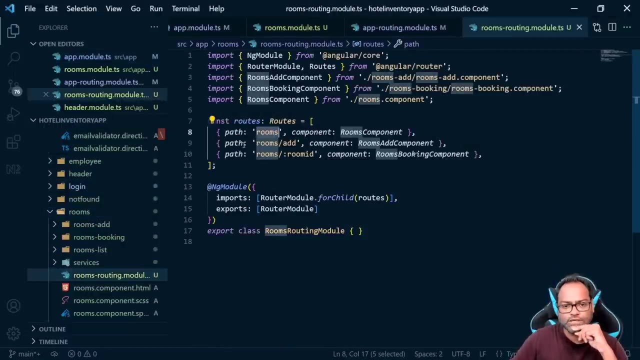 You don't have the form. of course, we will add the form later on, but let's try to fix. let's try to build this scenario using the nested routes concept. Let's go back to our code. let's see where the routing exists. so our routes are here. so what we want is this room: slash, add should be. 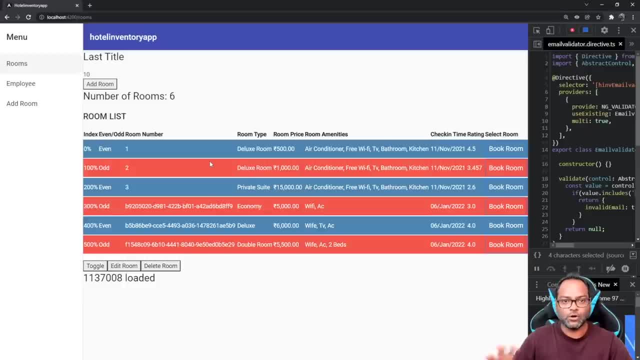 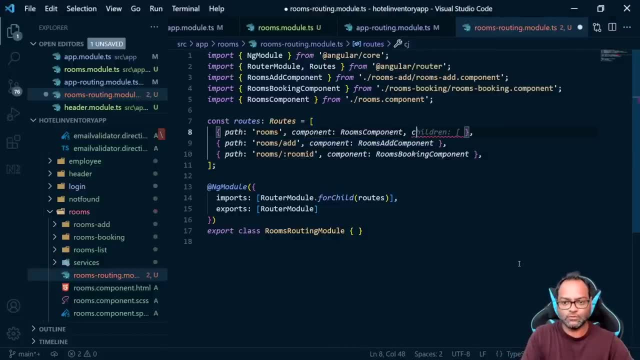 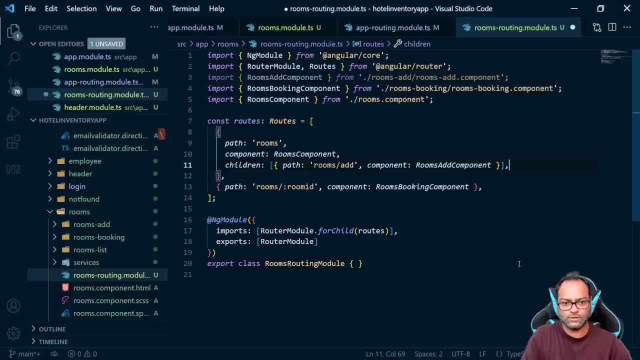 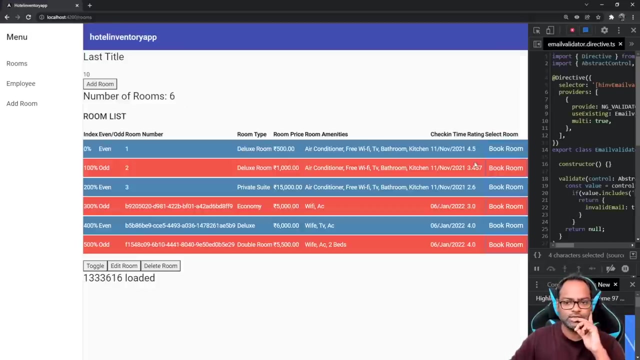 Loaded on below- sorry, not on, but below- this particular table. So we can do that. So here you can use something known as children property And you can move this route inside this children property. So this is step one. once we did, we have done this, let's see. 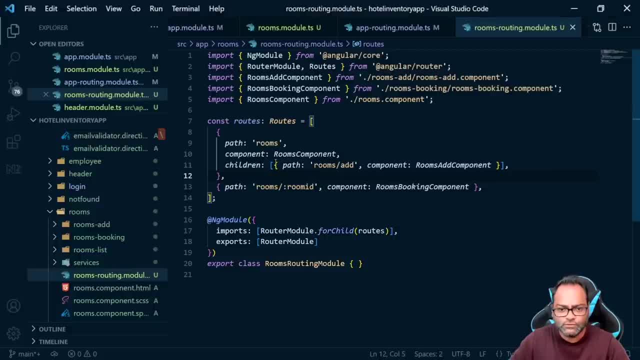 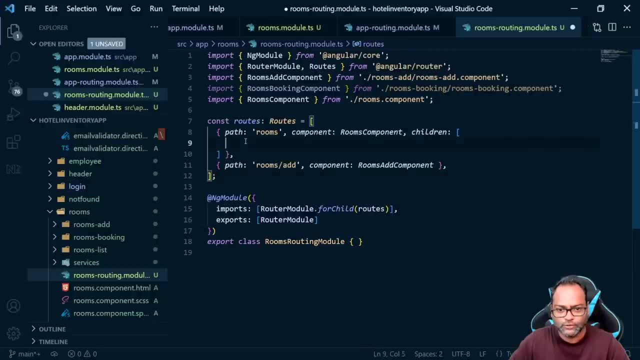 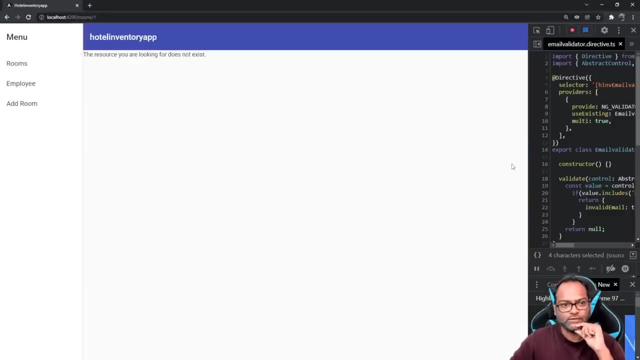 Right. I mean it is getting loaded on another view Because we are referring to the wrong view altogether. So this is the path which we needed: room slash ID. Now let's go ahead and see. Yeah, you can see. when you click on this, it goes to this room slash one, but it says the resource you are looking for does not exist. 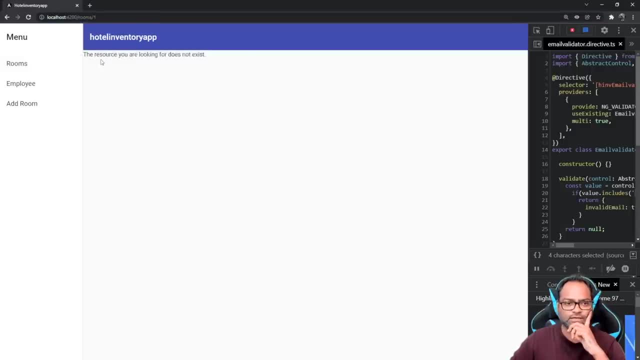 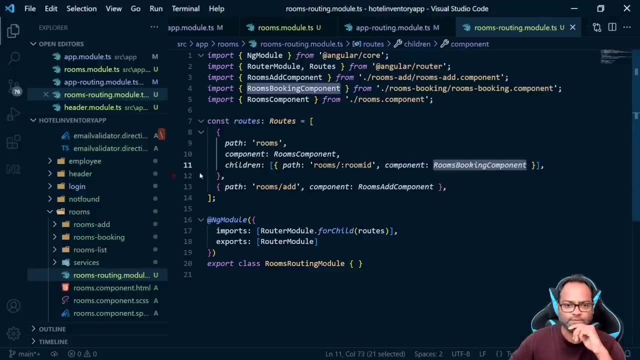 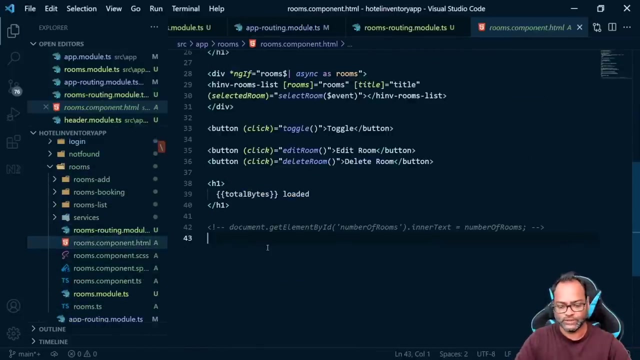 This is strange because we said room slash ID is already configured And it should go to Rooms booking component, but this is not happening. So now we have to do one more thing. We have to go ahead and tell where to actually load this rooms booking component by placing another router outlet. 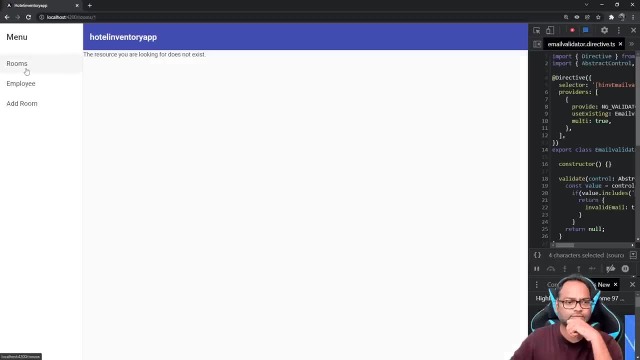 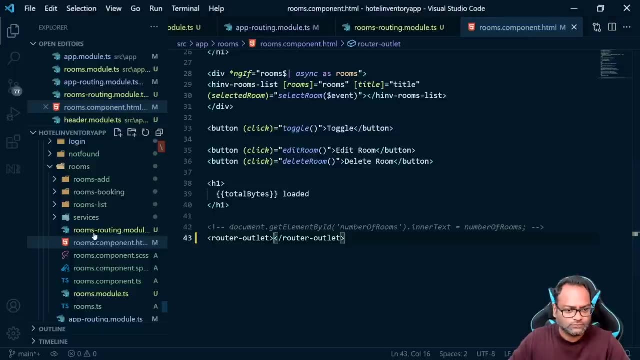 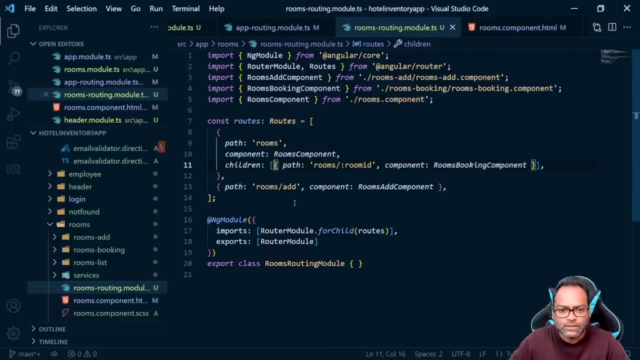 So let's see how it behaves now. So let's go to rooms. Let's click on book room, Let's see What's different here. Okay, So now, as we are already inside rooms, so we have to remove this. 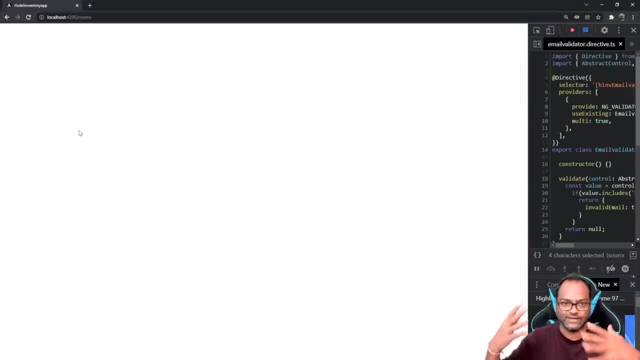 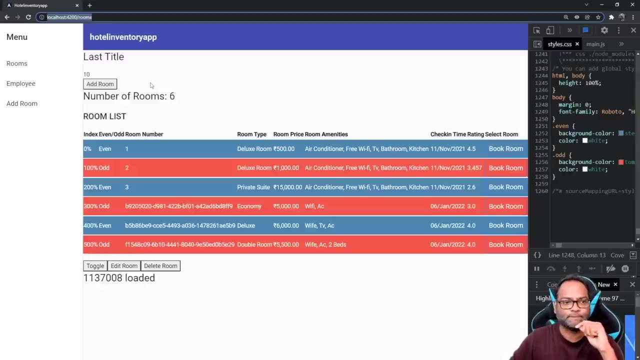 Okay, Let's see rooms. So, because it's child, right, So it's child route, So we have to remove this last as well. Now let's click on rooms and click on book room. You can see this component is actually getting loaded here. 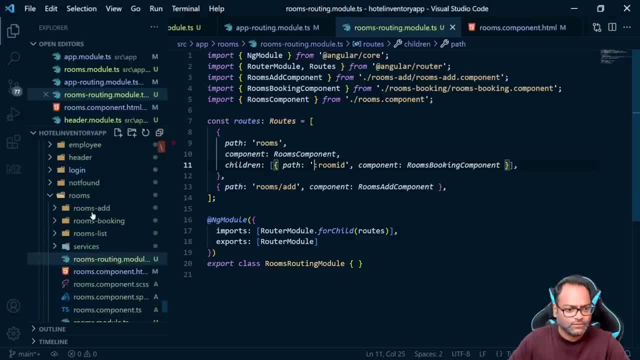 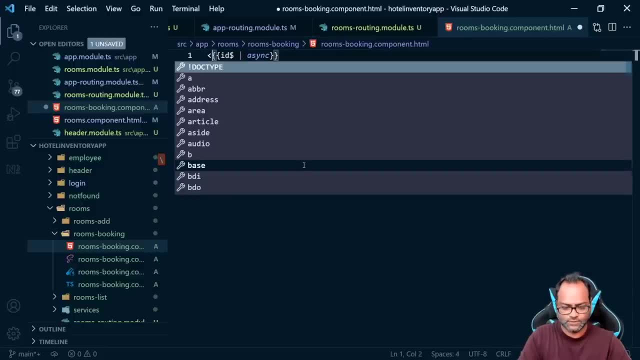 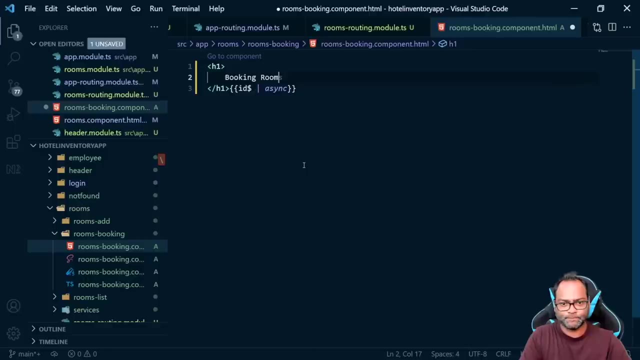 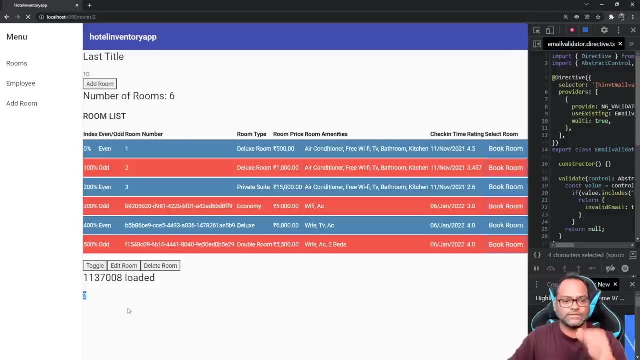 Let's put some more content here. So I'll say booking. So this is H1 booking room, So it is visible, right, So you can see. So, booking room. two: click on any room you want to book and it will be displayed just below the table, wherever you have placed the router outlet. 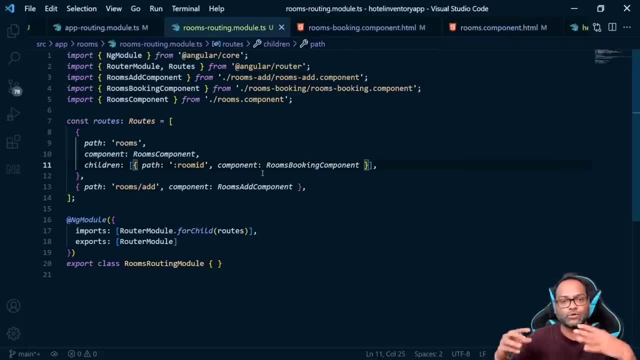 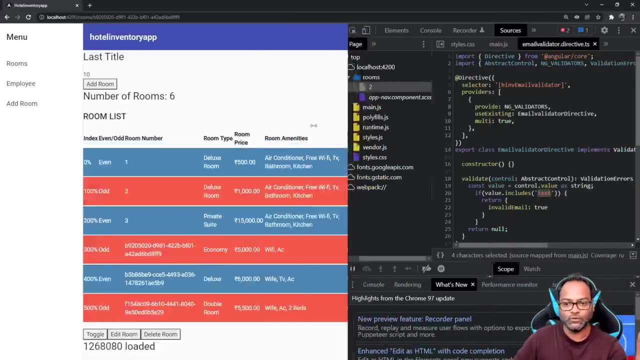 So remember two steps. Two steps which is needed in case you want to do nested routing. So why it is nested routing? Because you can see this is already available inside a router outlet and then we are loading another router outlet here. 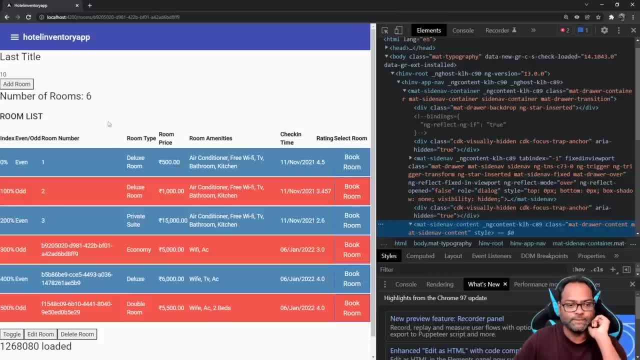 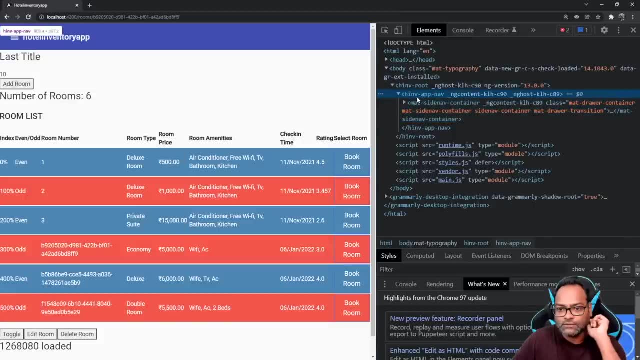 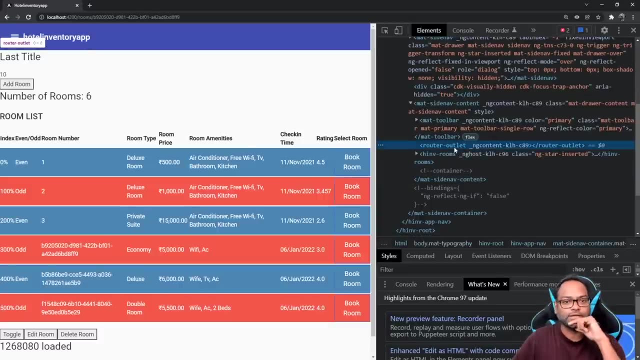 So let's try to understand this template right. So here we can see this is our first app. and then you have the sidebar and we have first router outlet here, Okay, And then there is another router outlet which is available here. 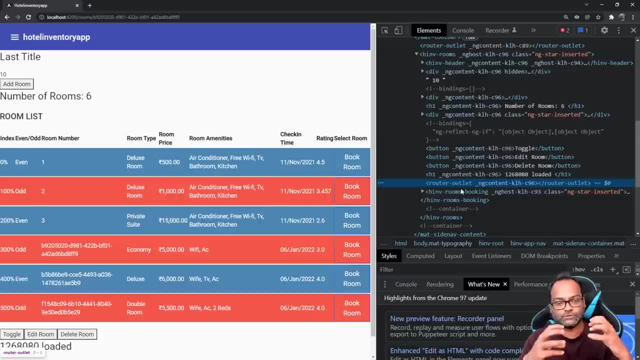 So it is nested right. So understand the nesting. It's one thing, same thing, again available inside the same thing. So router outlet, again available inside router outlet. That's nesting And as it is getting loaded as part of this existing component, it is treated as a children routes. 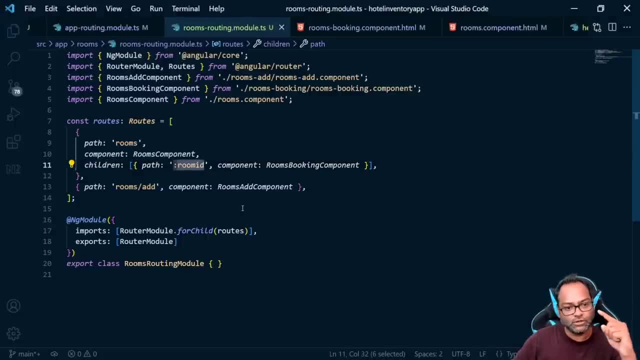 So you can see this is children. And then we are saying when we click on room slash ID, So we don't, We don't have to specify room slash ID again, here We can just say colon room ID and that particular component will be loaded wherever we place this particular router outlet. 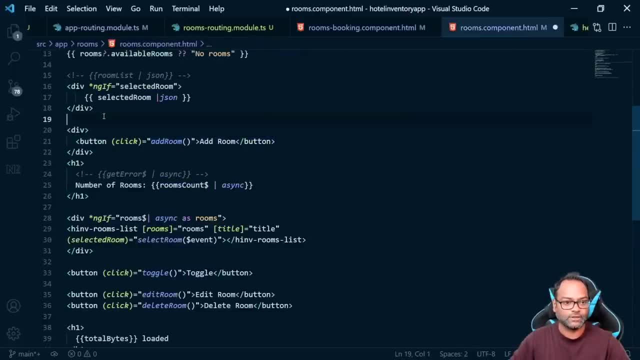 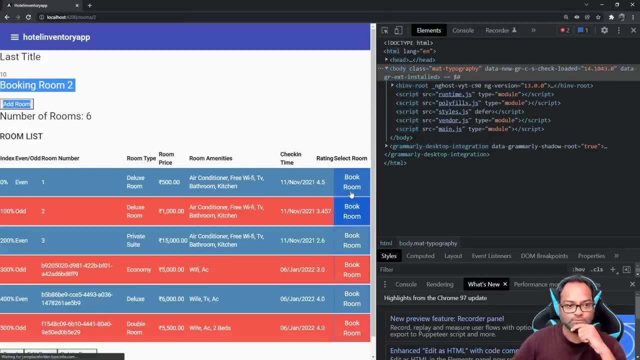 So if I place it above here So you can see booking room, this one right. So whatever room you select, it will be loaded here. So this is how you can achieve nested routes And Children routes. You can play more. 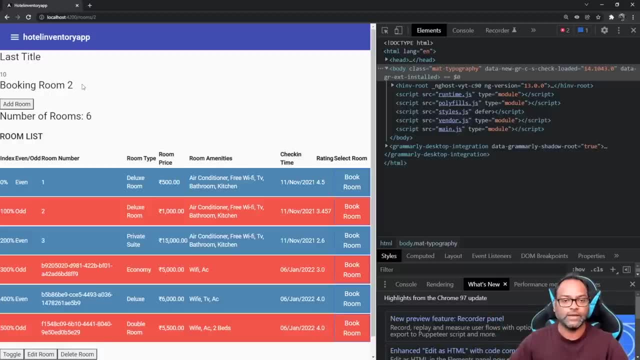 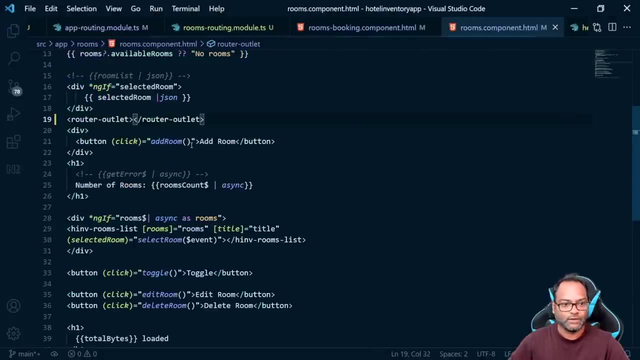 I mean, you can actually experiment by creating more child component and see how we can load them. You can load multiple, So it's not like only this will be loaded. You can actually add multiple here. I can just do, I can. 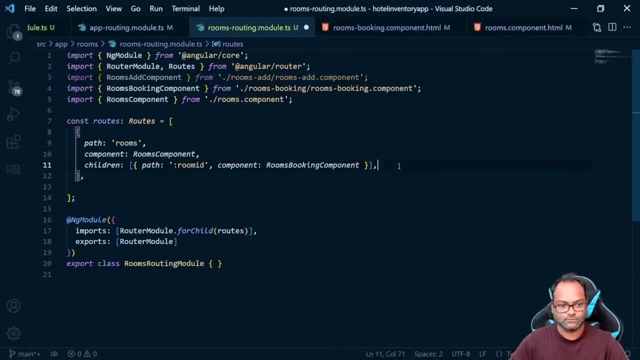 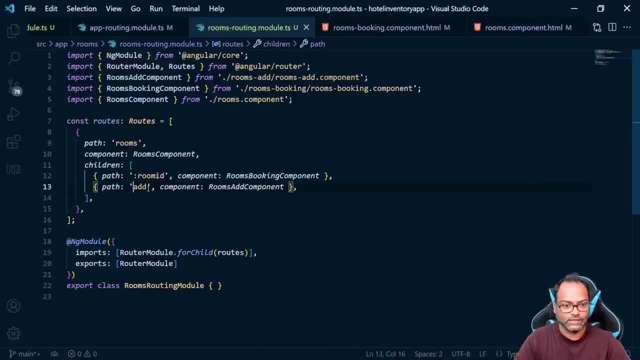 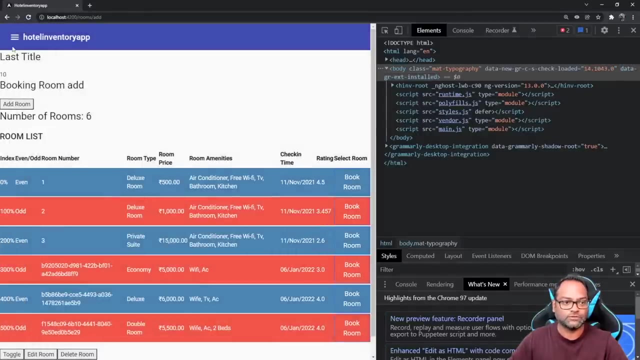 I can also move this one Right, So So, So, inside this, Sorry, And I can remove this and I can say slash. So now it is also child component, So the only thing is actually, ad room is available here. 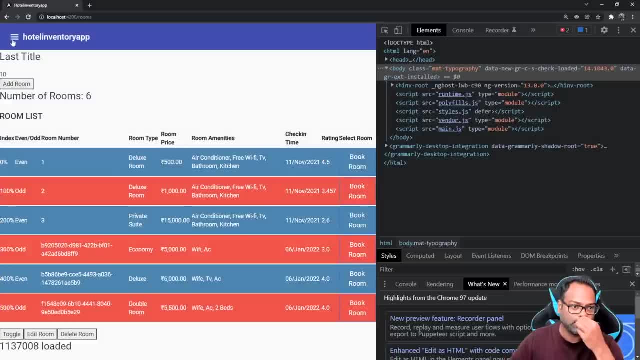 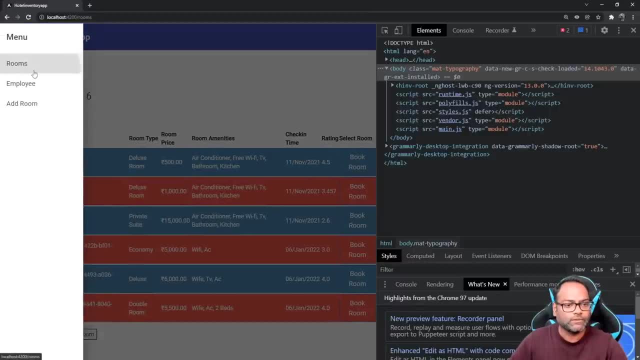 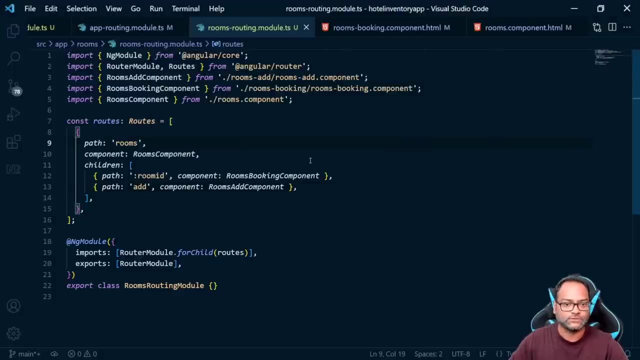 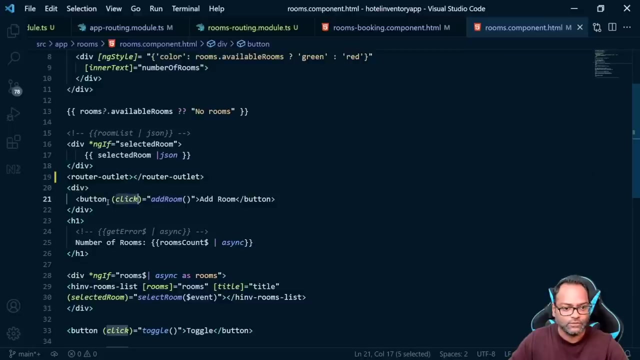 So if you try to click, So let's go to room And let's click on ad room, You can see, Let's, Let's do it on this one. let me just do this. and here on rooms, component of html, on add room. this one, right, so on add room. 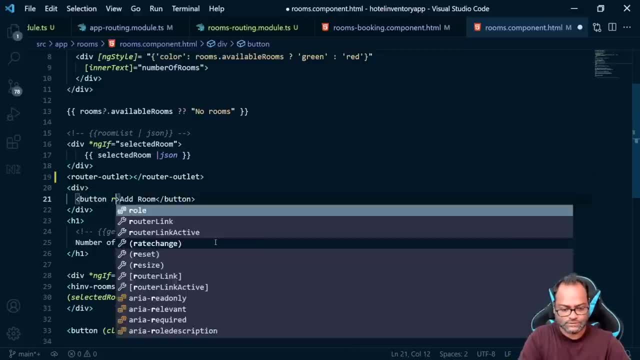 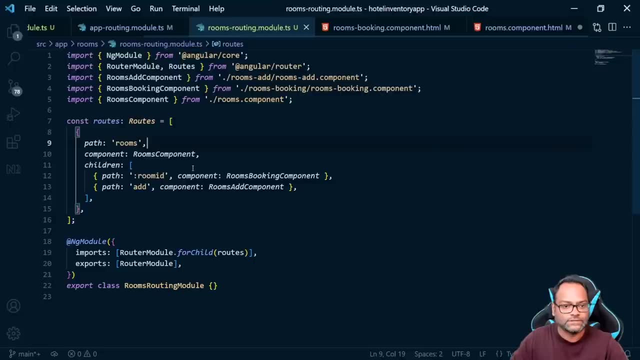 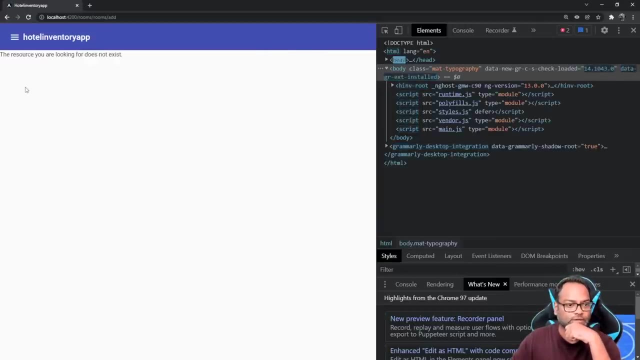 let's do router link. so we'll say this is router link and i'll say this is room slash add. let's verify if it is correct: rooms- okay, it's rooms slash add. and let's try to add a room. let's click on add room and it says room slash- room slash. 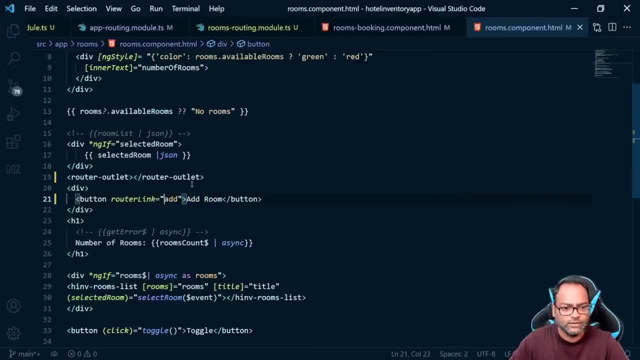 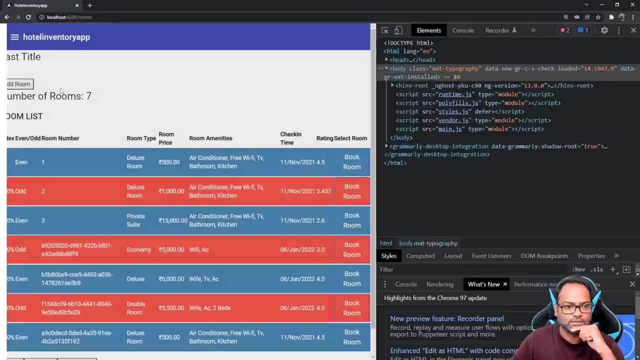 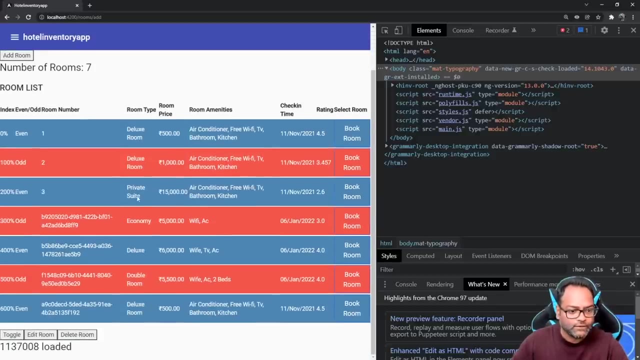 add, the reason being because we are already here. okay, let's see, as we are already inside child, probably that is the issue and here it is all right. so we click on add room and booking. uh, and what is there? inside room add rooms add. okay, this is the form. room slash add. where is this form? 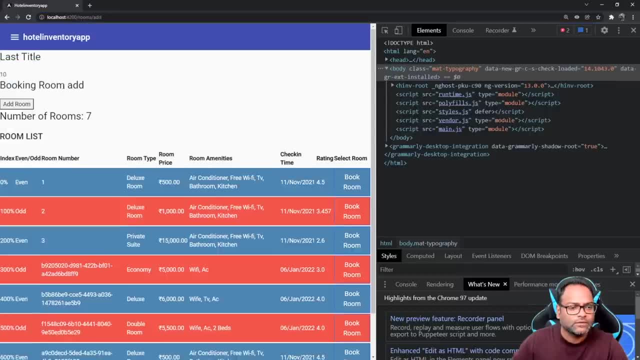 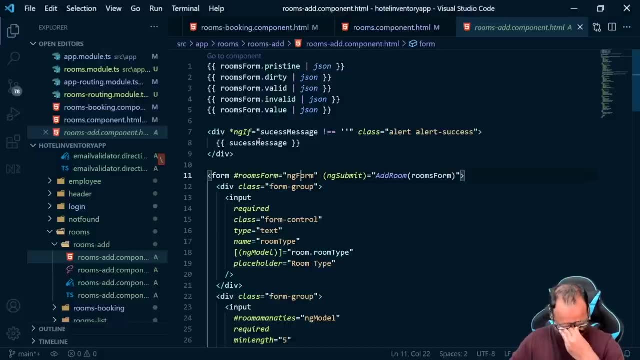 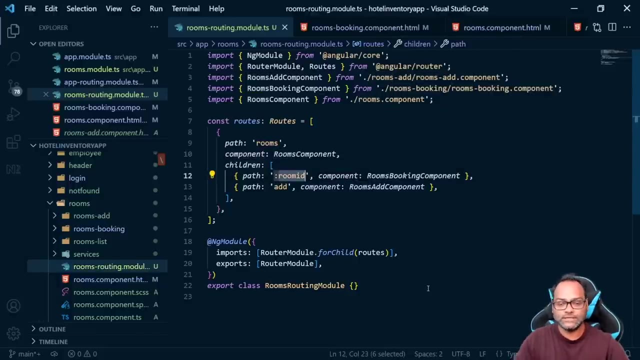 gone. okay, okay, booking. okay, this is good that we came across this issue, uh, here. so, uh, the thing is right now. uh, if i say room slash room id or i say room slash add, this slash add can also match to this the reason being it. uh, it's like it just uses that, okay, i, i can say room slash any placeholder. 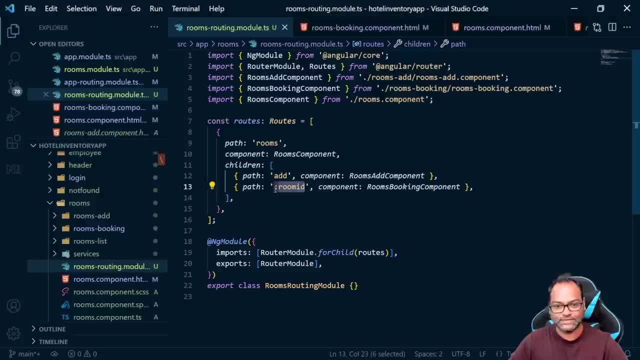 and this will be called so to avoid this, just make sure that, uh, you place at this, uh, this before, and then you have dynamic routes after this. that's a really good thing that we actually came across this issue, because this is also one of the uh reason where a lot of developers get stuck. 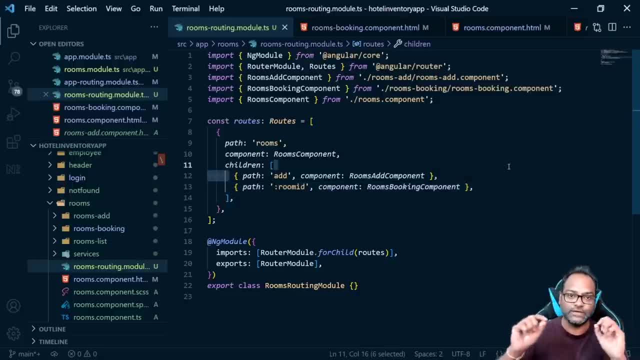 so what we have done is we are saying that add is first, so it will match to add. but if we place this one, i mean it's a wild card, right, i mean it's a, it's a placeholder. so if i keep this first, it will also match to room slash add and it will always go to the booking component. that was uh. 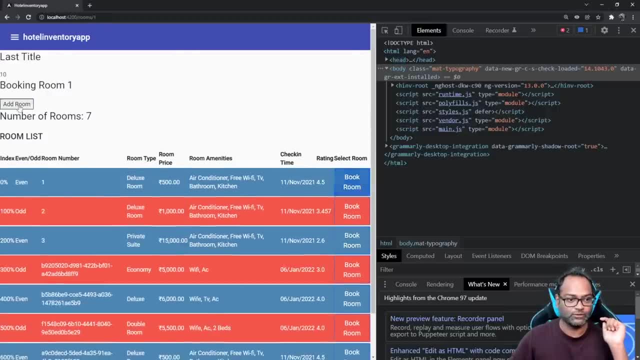 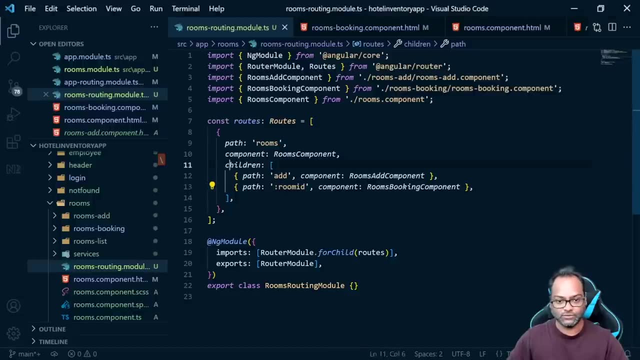 the thing now. if i click on book room, you can see i'm getting going to this. if i click on add room, i can see the add room functionality available on this view itself. so this is how you can play around with multiple children components. you can add a number of children components in case you 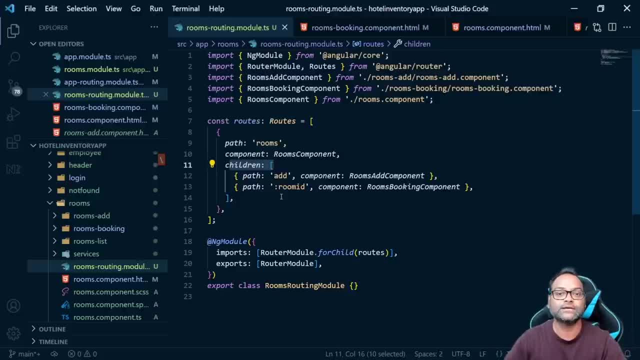 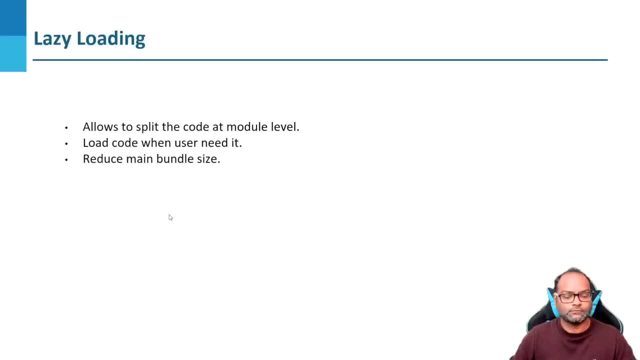 want to display them on the same view. you don't want to redirect to something else, so you can do it somewhere else. so this is how you can do it, and let's move. so far we have seen how angular routing can help us to create several routes, and in last video we 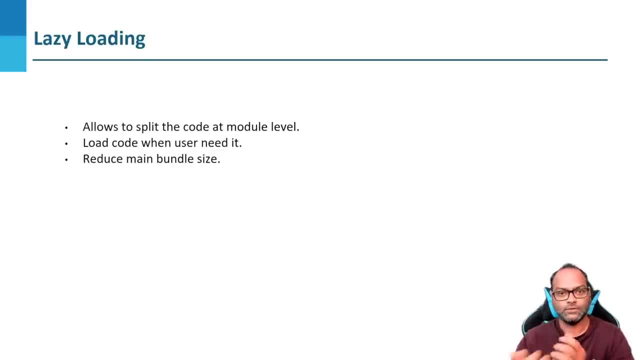 also learned about how you can create modules. so, as discussed, modules are something which where we can actually wrap all the functionality related to a feature into its own module, right in its. but once your application grows, there will be many models and so the application size will grow as 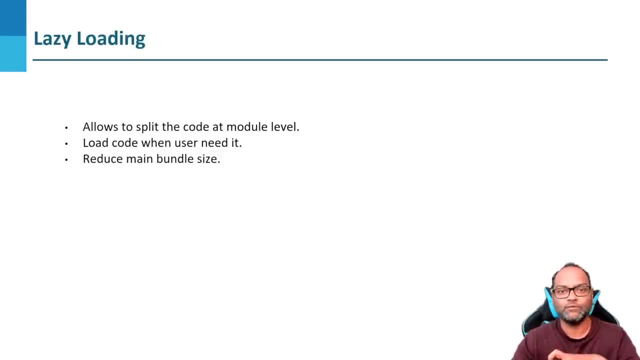 well and one point of time you will probably end up with huge main bundle size. so this is where we will talk a little bit about the build which we create for deploying on production. so so far we have been using a command called ng serve, which is used: 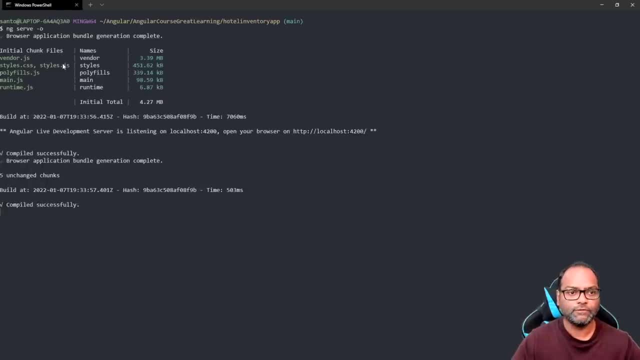 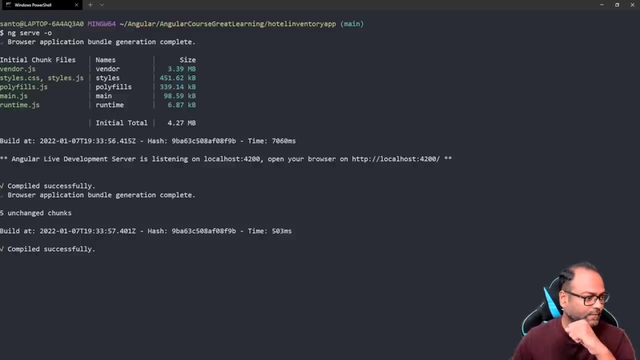 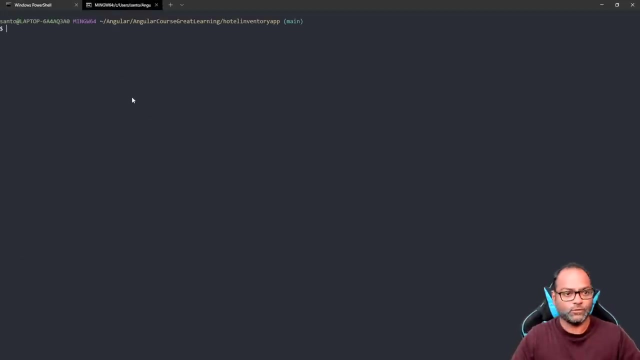 to run this application locally and debug it. now we will use another command to create a production build which can be used to deploy your application on production. so to do that, i am going to run a command called ng build and you can say: i can see equals to production. 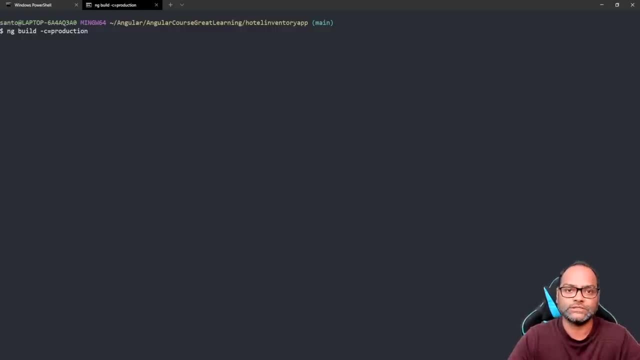 now, what this command will do is it will build your application with production mode. so this, this, uh, whatever files which will be generated, it will be minified and it can be deployed on your production server. so let's see, it will take some time to generate the bundles. you will get several files and we will talk about one main file which 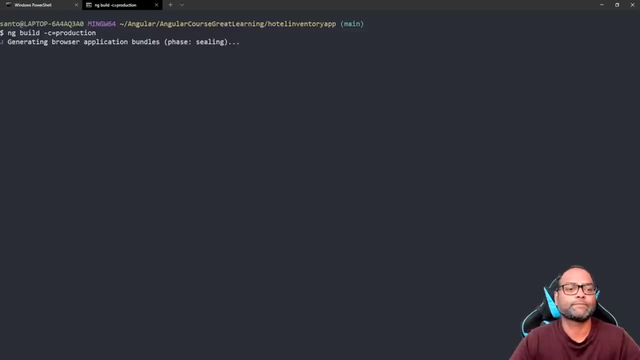 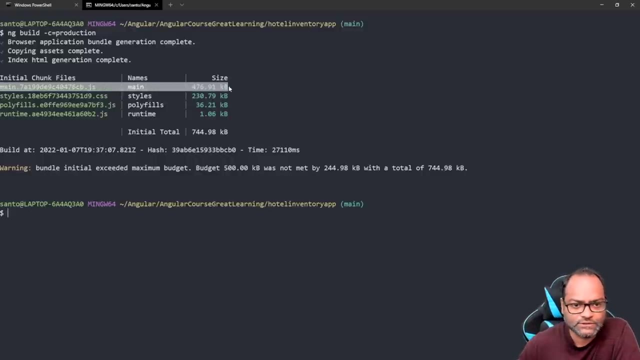 is called mainjs. so here you can see, uh, you have mainjs, which is around 476.91 kb. right now. our application is really small. i mean it uh. it contains an app, modules, a few components and one module. consider it like a huge enterprise application. 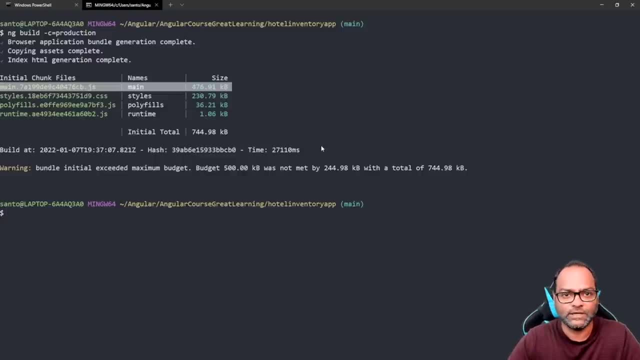 consider: uh, now, in future, you will end up with a huge enterprise application you are. you will probably have hundreds of modules. you will have thousands of components, even not that big, let's say in range of 100, right, so this bundle size will increase and this mainjs. 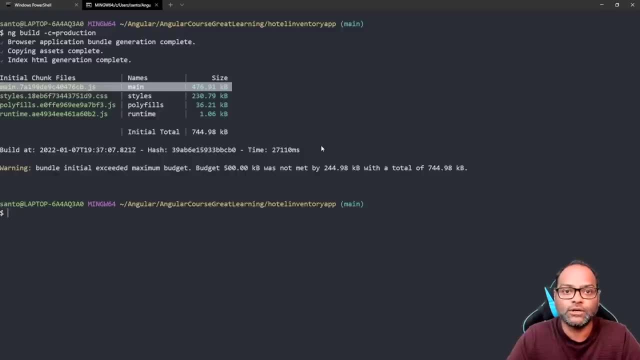 is the file size which will be served to your customers now. 476 kb is it's okay, right, i mean it can. it will be pretty fast on your 4g network. but what in case? you have this bundle size in mbs, and that's where the problem comes in. now you will have 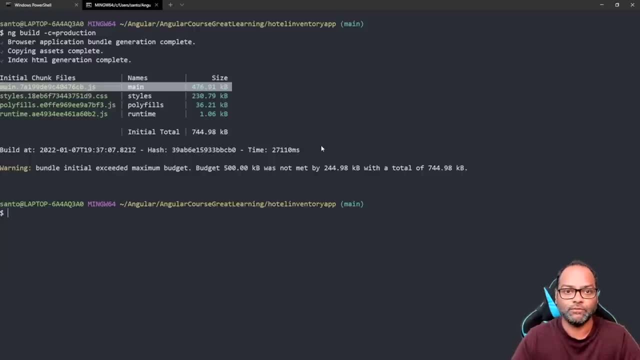 a big bundle which needs to be loaded whenever your, your user, comes to your portal. so they have to wait. they have to wait based on, uh, how much speed they have right, how much the bandwidth they have. what you can do is using angular mod, angular router. you can also split the code. 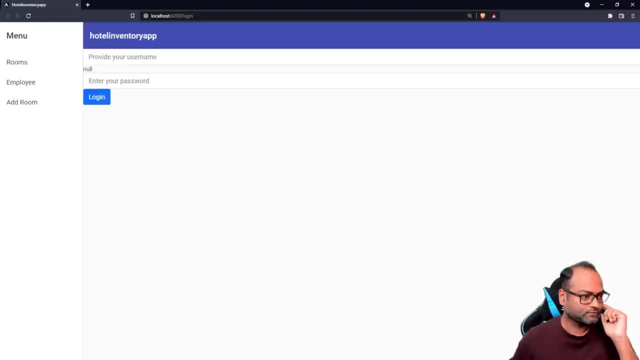 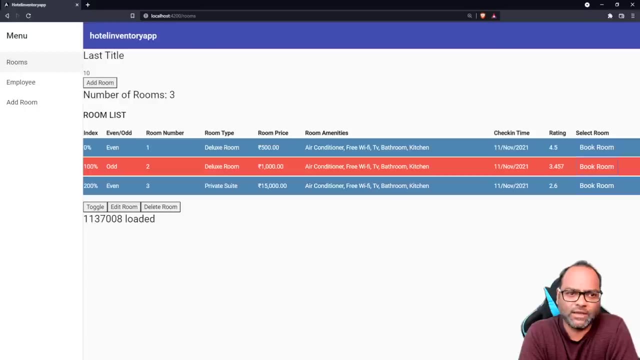 if let's go back to our application. so if you see here the functionality related rooms, do we think i mean this room's functionality should be available by default to the users? the answer is no right. i mean, of course we, we have to actually go ahead and add few. 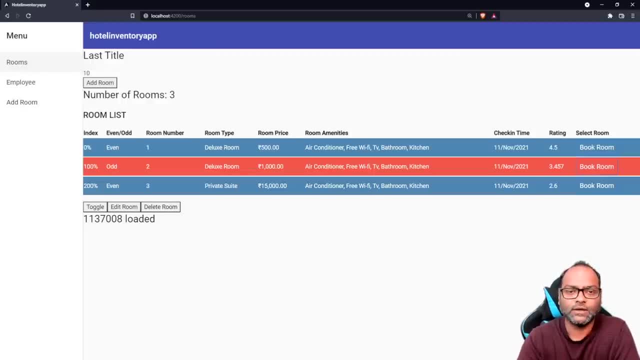 forms, more functionality to our uh, to our login screen, and that will be the first page which will be served to our customer. so without login they cannot even use this room's functionality, even employee functionality. so it doesn't make sense to actually give all this views with. 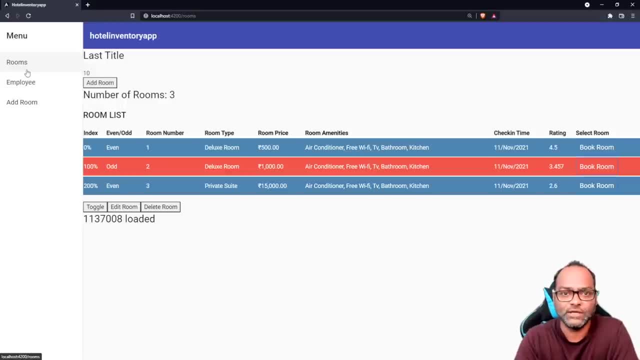 your mainjs bundles. i mean, all this code is something which is used, as at that time, probably, your user just comes to login page and goes away and this, this code, will never be used. so this is where actually angular router can use. angular router can help us to split our 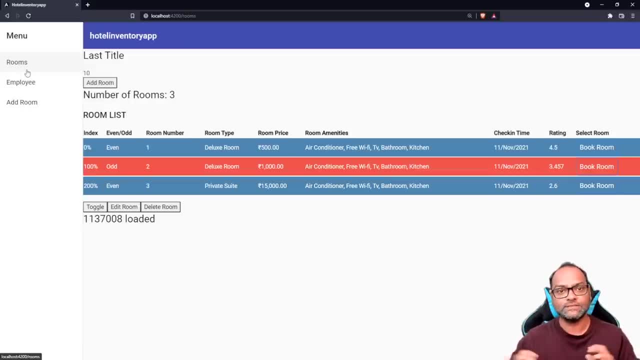 code based on several routes. it has some advantages, of course. uh, this code will never be downloaded, in case your user never comes to this particular route. and once the user visits this, it will be once. it will be downloaded only once. so it's not like i mean, if i just go to 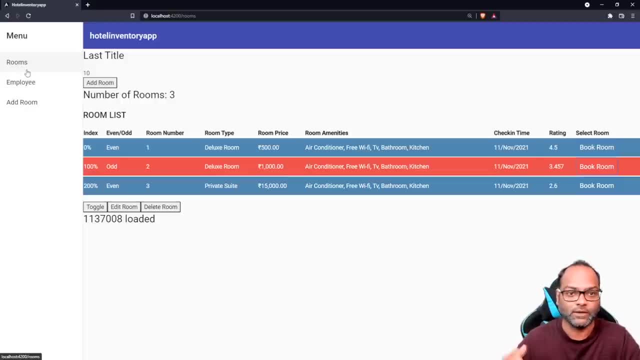 another route. this all code will be um removed and then will be added back once we come back to this route. that that's. that's a no so? but there are few requirements which you have to fulfill to achieve this. what are those requirements? remember, whenever you are trying to create a 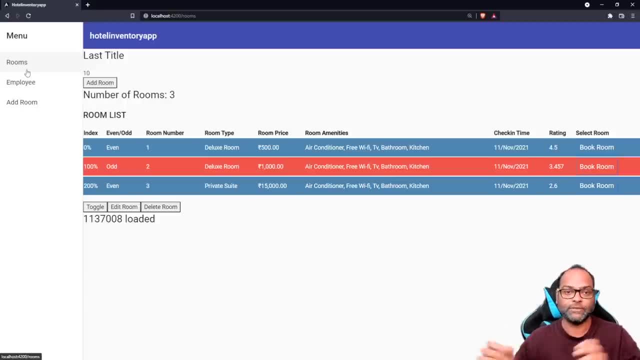 module as lazy loaded model or you are trying to separate that code from all entire application. the first thing which you should think about is: what are the things which needs to be reusable? if it's reusable- probably you have- you have to rethink about your architecture. let's say there is one component which is reusable from rooms. 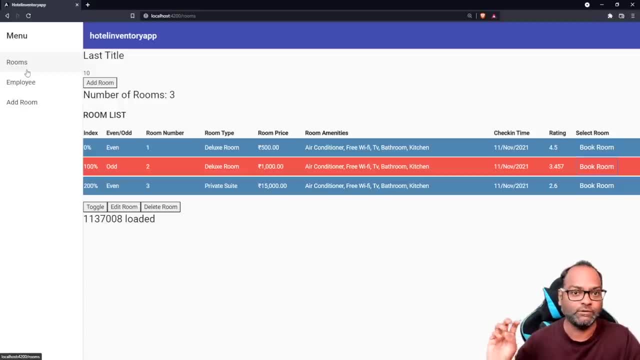 in that case, i will remove that from the rooms component. i will put it somewhere else, which is where we will put reusables, so i can use it inside rooms and other places as well. never do something like this where you have rooms module lazy loaded and then you are, there is one component which is being used somewhere else. 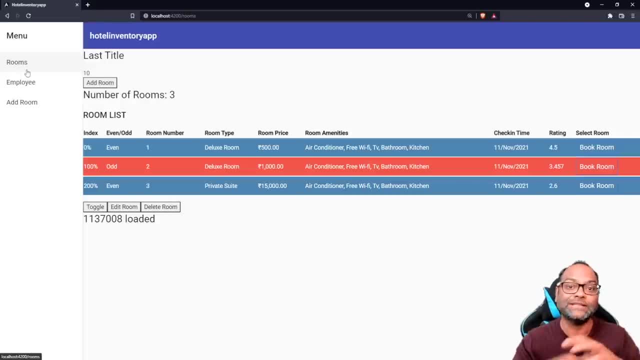 in that case you have to go ahead and import rooms module in that particular module, which will fail the purpose of having a lazy loaded module. so a lazy loaded module should be isolated. i mean it should not talk to any anyone else, it should know everything about itself and once loaded it should be able to perform all the functionality and your 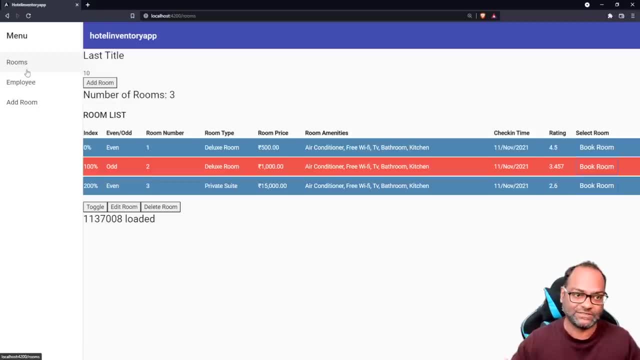 application should not know about this module until unless it is requested. so here we are talking about: this code will be downloaded based on user interaction. so once i interact with this rooms module or rooms url, the code will be downloaded. so let's go ahead and see what are the prerequisite. 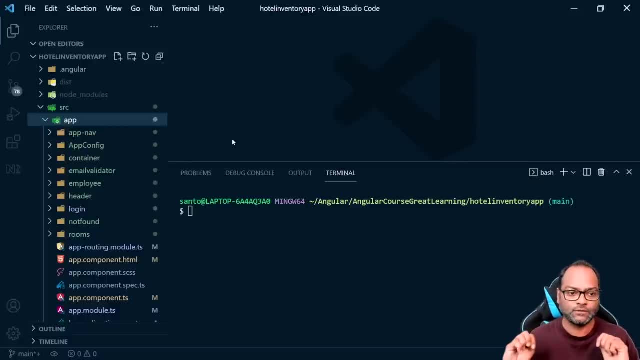 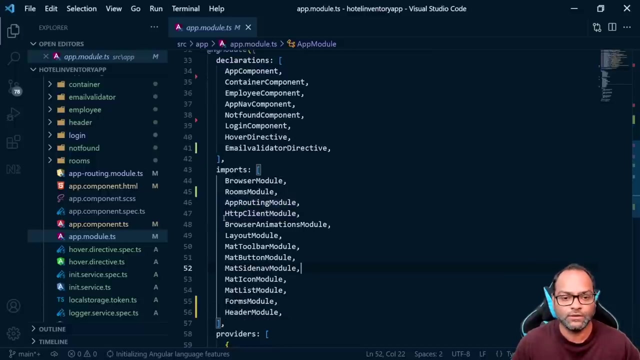 so first thing is now, as we have chosen the rooms module to be lazy loaded, the first thing is: no one should know about rooms module. remember last time. what we did is we created a feature module for this rooms module and then we added here. so first step: remove this. 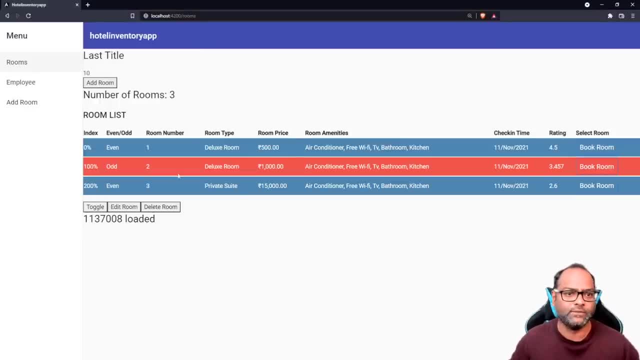 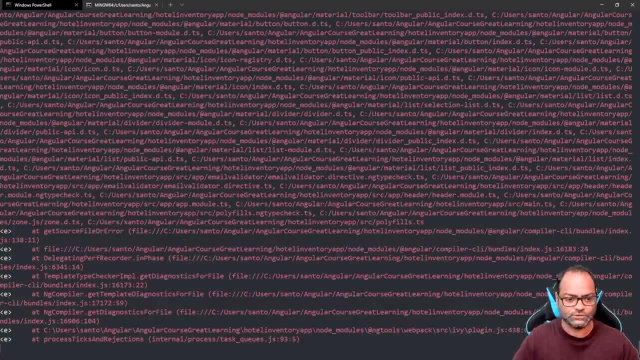 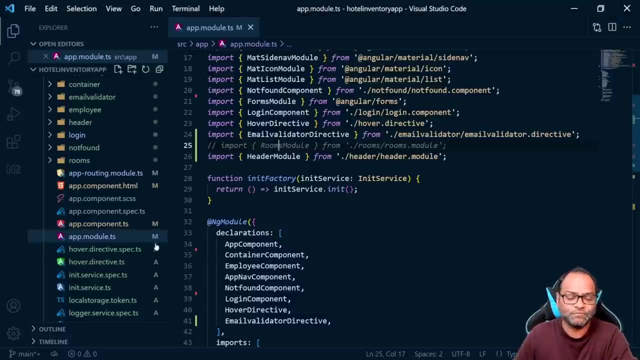 now no one knows about rooms module and it should not work right. i mean, if i recompile the application, you can see there are a lot of errors because, of course, release this, rooms module is gone. i mean, no one knows about rooms module anymore. now, what's next? now here in app routing module, we will add one part. 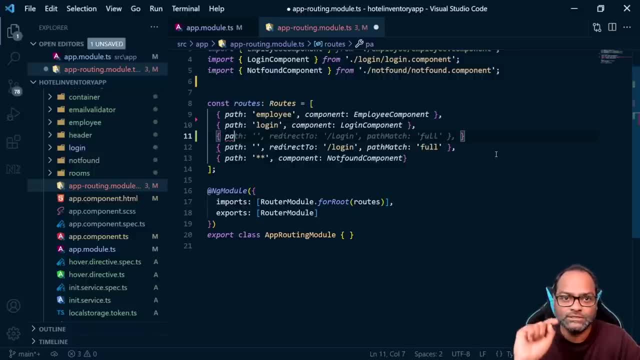 remember we have already fulfilled one particular step. we have already isolated everything related to rooms module in its own module, so we are not sharing anything outside rooms module, right? so just keep that mind, keep that in your mind whenever you are designing uh, this lazy loaded uh module for your application. just keep this in mind. here i'll say path rooms. you might be wondering. 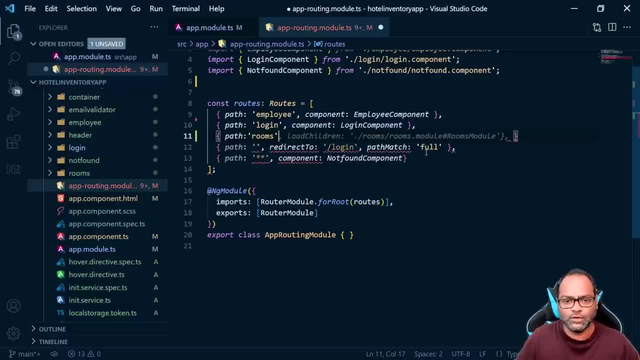 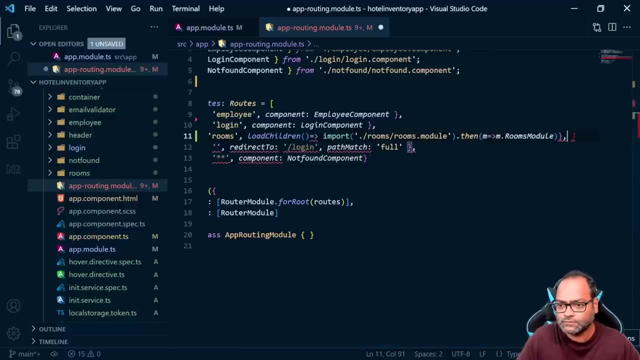 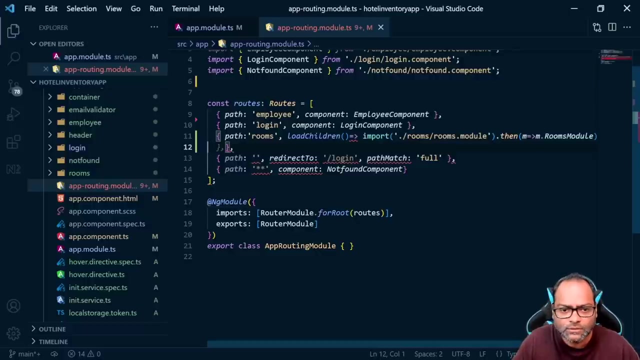 why we are doing here- and we'll talk about it- so uh, rooms, and then you have to use a property called load children and here we'll say you will be using an import statement. so i'll just let me just talk about this and, okay, something is missing. what? 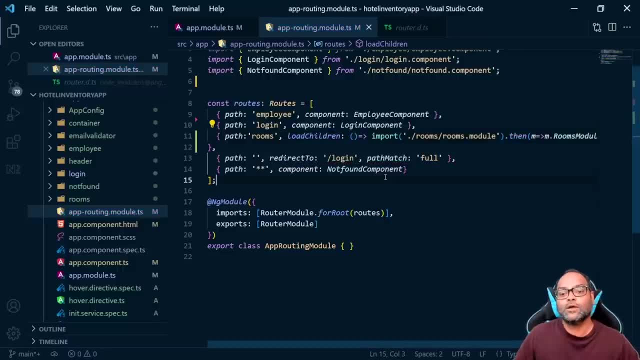 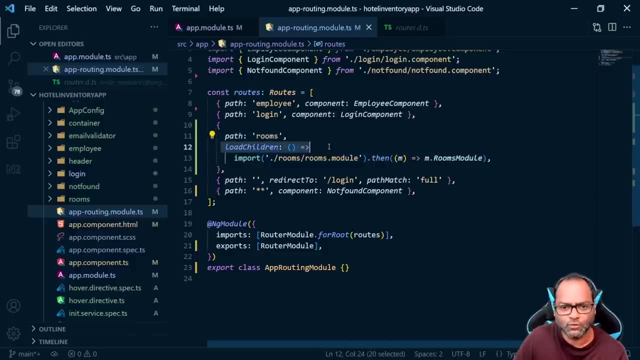 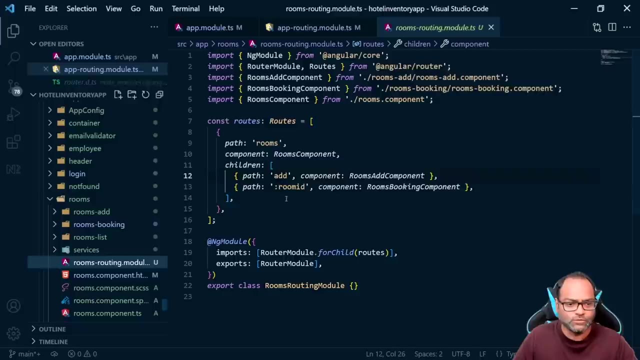 oh okay. so what we have done here is we have added a path- rooms- and we are saying: load children and then some import statement. we'll come back to this. let's go back and make some changes to your rooms routing module. here we will remove this path. we need to book it, put it blank and 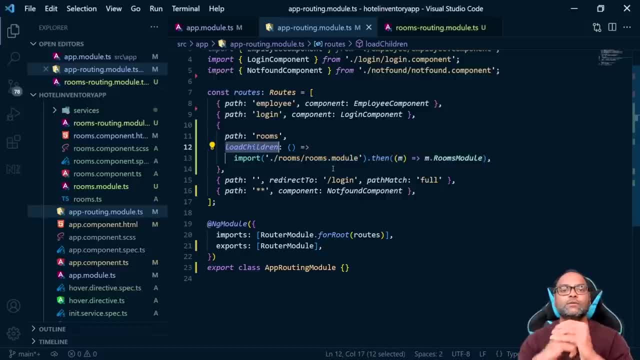 let's go back. let's go back and talk about this. so now we, rather than actually directly importing the rooms module into app module, so what we are doing is we are trying to lazy load it. so the lazy loading means now we are providing the path inside the routes array, because of course, this is your. you remember app routing. 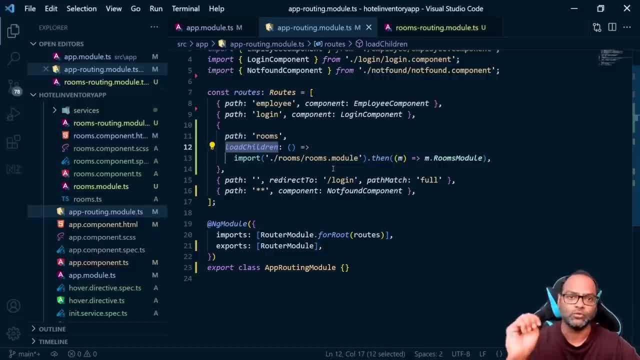 module, right, the main routing module. so now my app routing module knows that there is a path called rooms, and whenever someone tries to access rooms, what i have to do is i have to go ahead and download this particular rooms module. remember, this is the module which we created earlier. 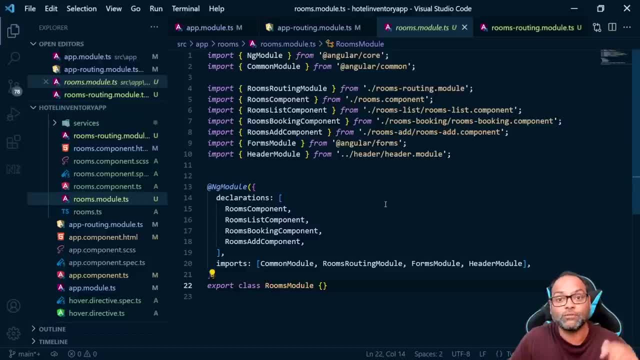 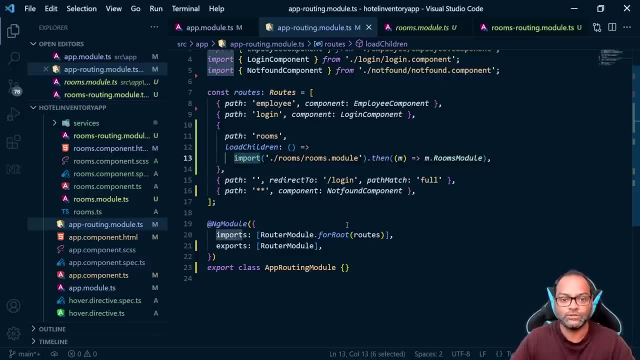 and download this rooms module, which has a angular model called rooms model, right? so this is this import statement is something which is native into to the browser. so at run time, at run time, remember, i'm not talking about the compile time. compile time is when we are actually building our 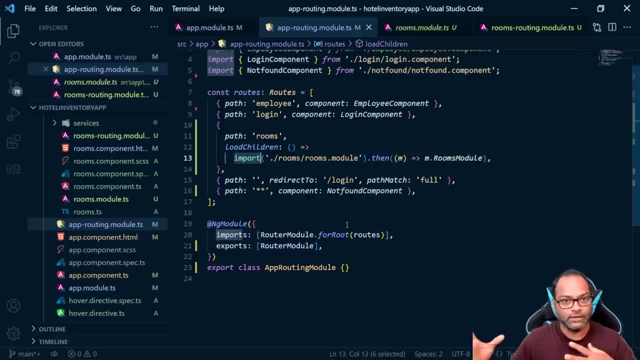 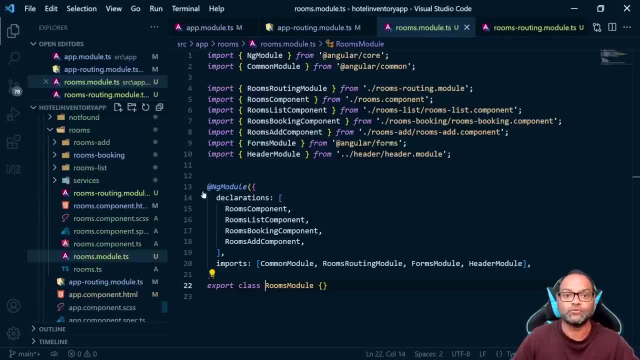 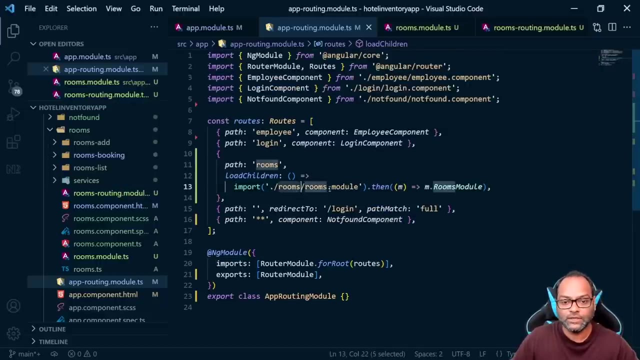 code right at run time. it will, whenever we click on rooms, it will go ahead and download all the code which is related, which is available here inside this rooms folder, and make sure that you are not using anything outside rooms module. right? so here we have. uh, we got, we did this, we can do. 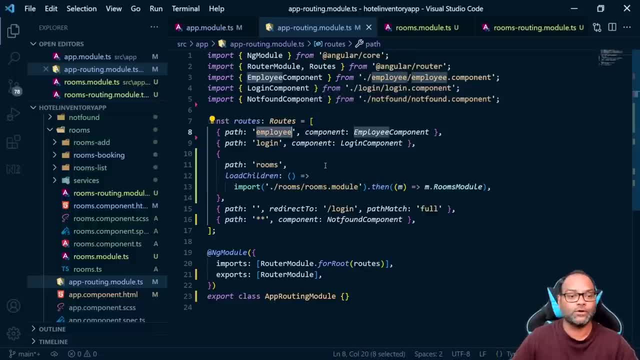 similar thing for employee. that's something which you can try. what you can do is you can create another module for employee and then try to lazy load that module. you have to just create a routing module and then you have to create a angular model, and those are two things which we have to do and then you can in similar fashion. you can. 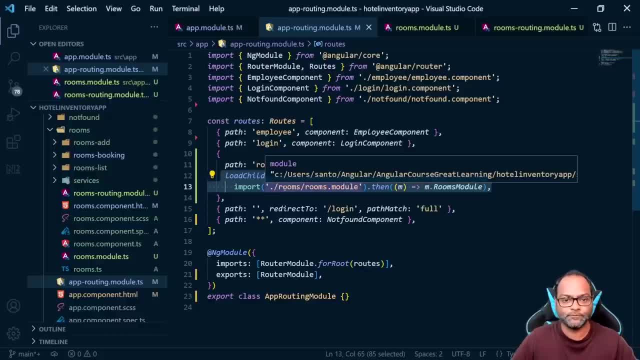 download the employee module. in case you are not able to do it, just raise the issue and we will help you. now this is also done. we have removed this because why we left this path blank? because we have already defined this path here. so when this particular module gets downloaded and it goes to its default url, i mean the first url, so it will. 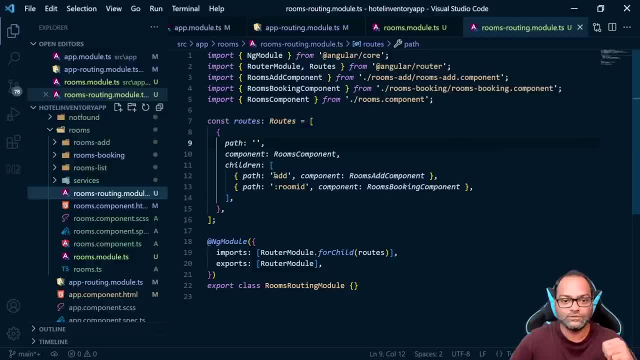 so when this particular module gets downloaded and it goes to its default url, i mean the first url. so it's a ά Passion of Modern alphabets framework, which is 부�Haðarj 볼ã goes in this name only and it will show you the seomat transitional Rail means all of the links between subscribe and 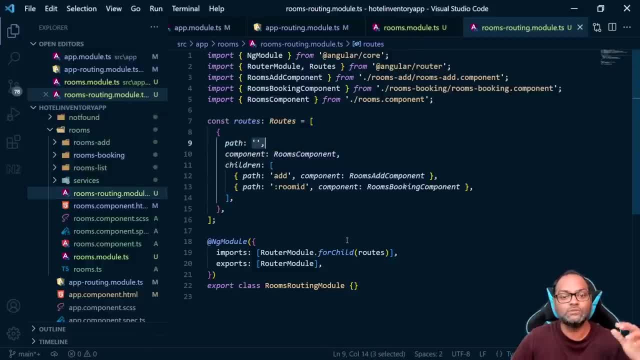 to always it. you can do this if you like. there's the link between subscribe and like bunny body, so it's a check. okay, this is the component which i have to download. so rooms is my default route. i don't have to do anything. and then we have the children, which we already configured last time. now let's go ahead. 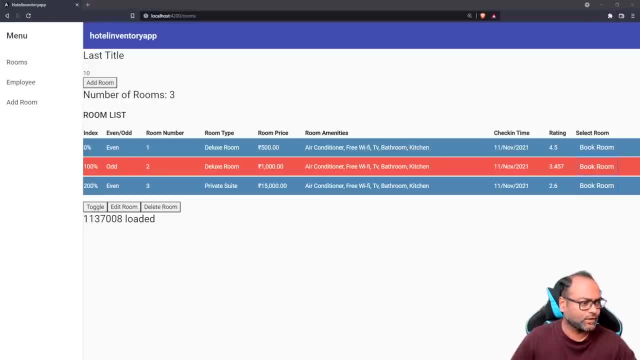 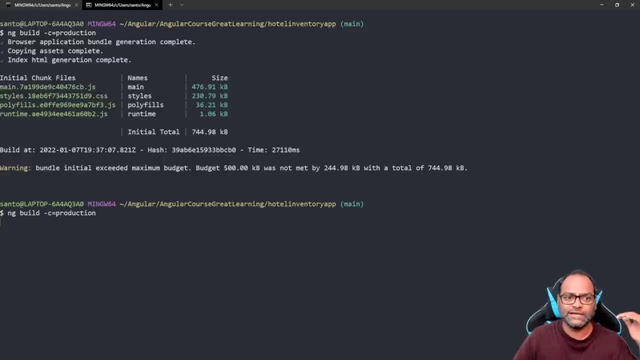 and verify the application. so two things we will verify. there are two things which we will verify. first, let's verify the build. let's see if there is any difference in the files which got generated earlier. right, so earlier we got four files. now let's see, uh, after making this changes how many. 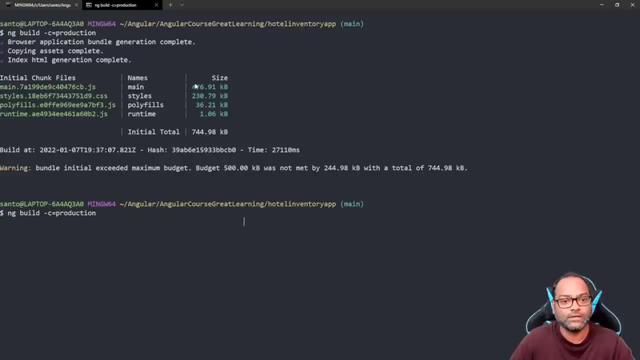 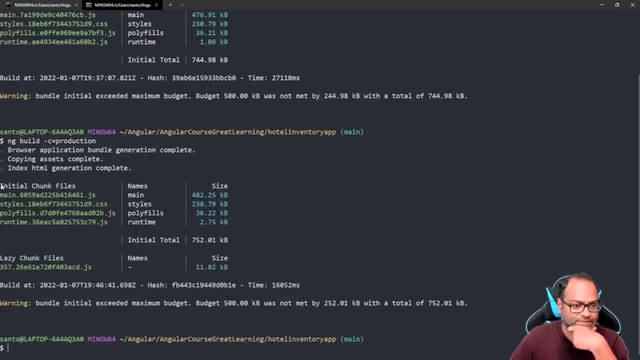 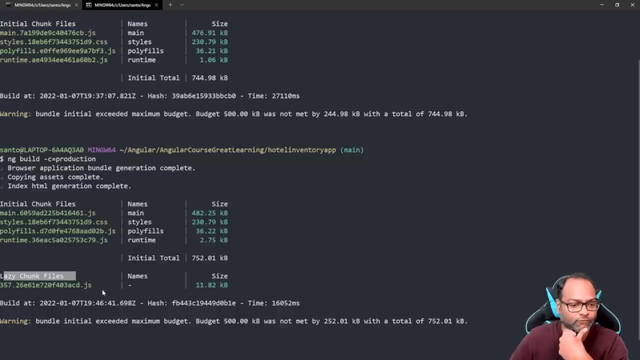 files we get and how it impacts- uh, impacts the bundle size as well. so you can see. it says there are some initial chunk files and there is something which is lazy chunk files. so you can see. now we have another module which is of 11 kb and 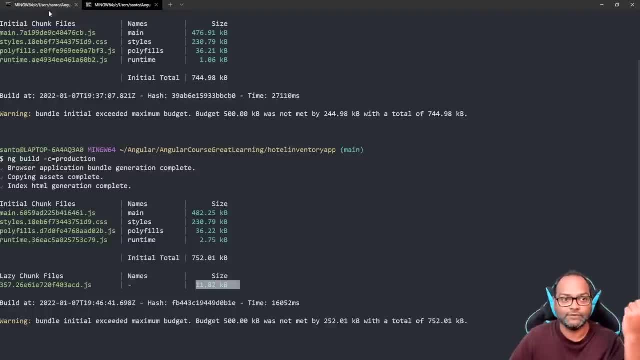 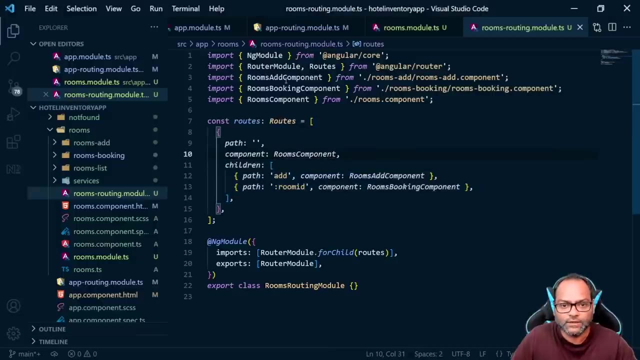 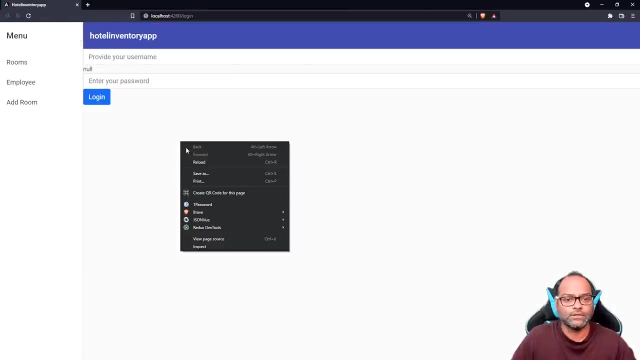 it will be downloaded separately once i interact with that particular route. let's go ahead and run the application now and meanwhile let's see if we are missing something here and okay, so let's verify how, if our lazy loaded module or lazy loaded functionality, which we did, is not 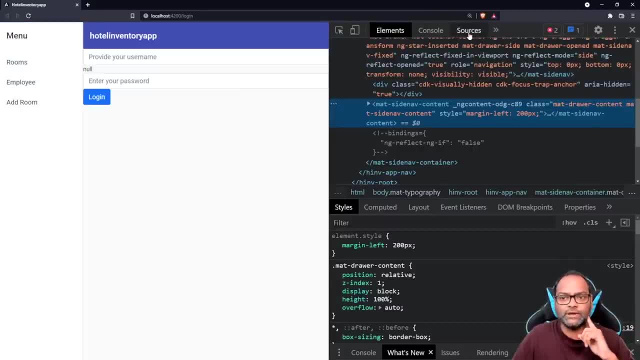 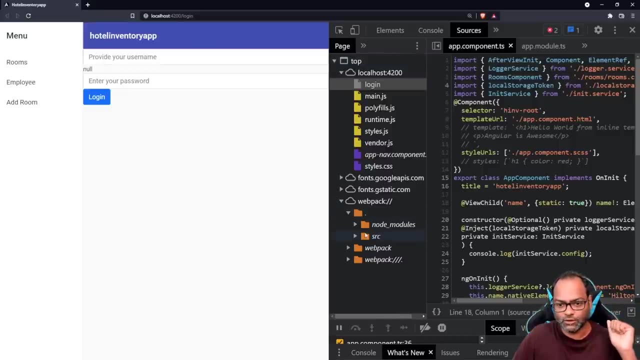 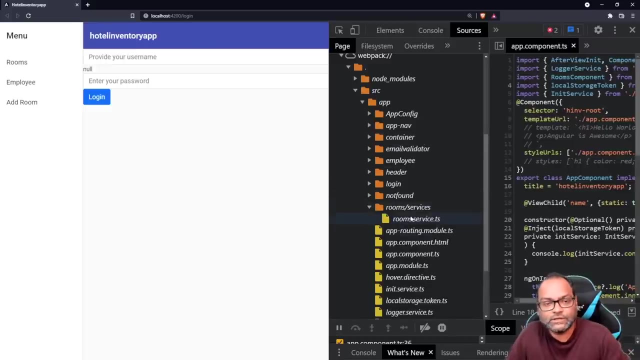 working fine or not, how we can verify. of course, in build we can see there was a different bundle all together, but we can actually verify it from here. so you can go to the sources, you can go to the pec dot and go to src app and here you can see. okay, so here we can. you can see we are actually. 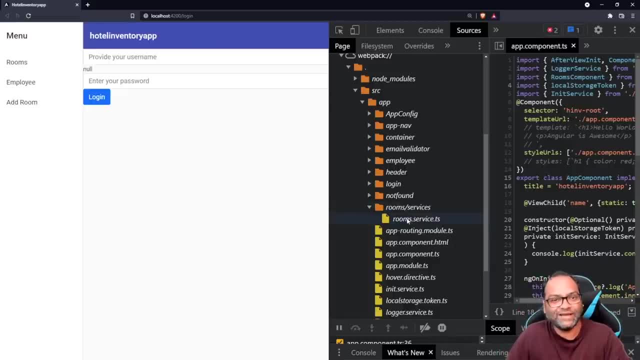 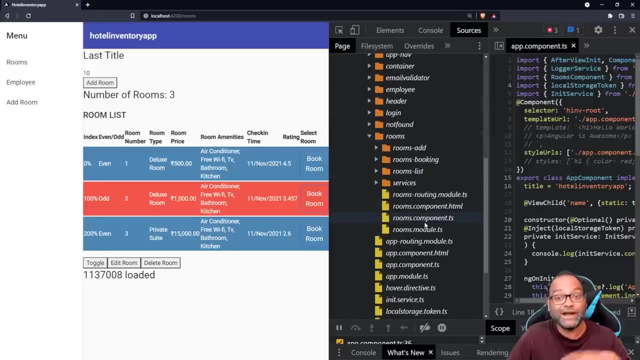 using room service somewhere, so one file is already downloaded because we are using it outside, probably, uh, in app module or somewhere else. let's see the main functionality. let's click on rooms. now you can see all the files, apart from services, are downloaded, as i clicked on these rooms and now i can just go ahead and visit. 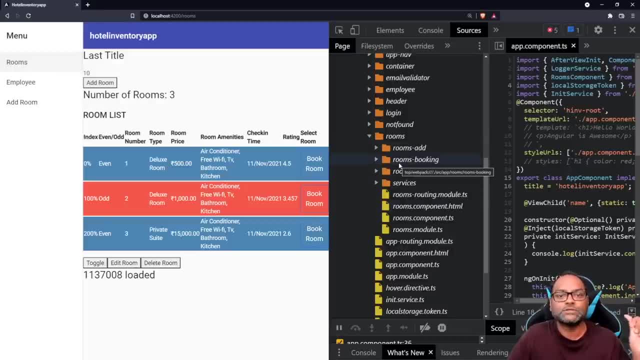 any other url that won't impact these files. so this is how you can verify what are the files which are downloaded. uh, lazily right, i mean, apart from services, everything is being lazy rooted right now, and it will be available as well inside your network tab, so let me just remove it. 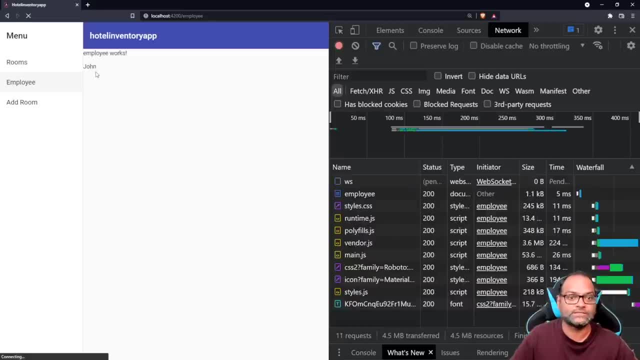 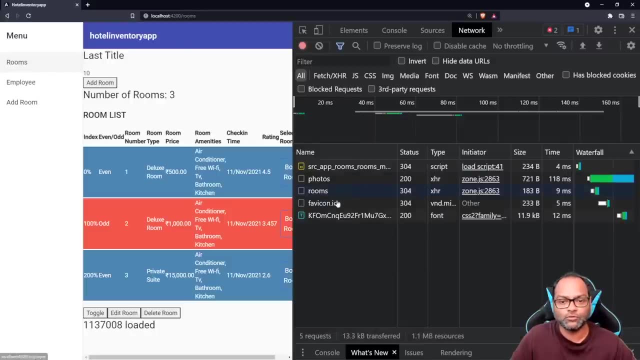 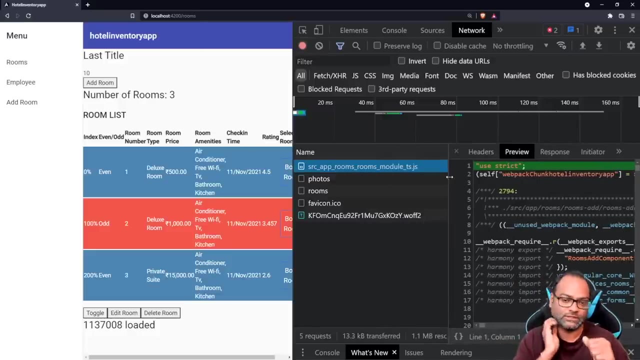 and let's refresh. uh, let's go to employees and let's refresh this page and let's clear and let's click on rooms so you can see src app- rooms- rooms module. so this is something which which is telling you that, okay, this, all the file, this code is actually being 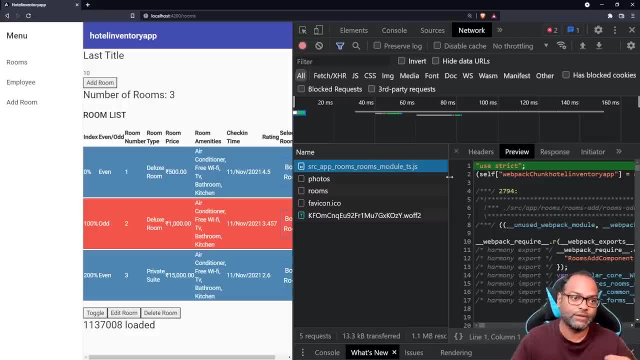 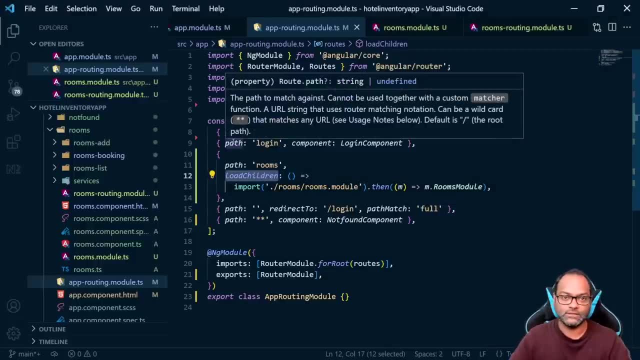 loaded separately and when it is happening when i click on rooms. so this is how lazy loading works and you should, as i said there are. there are many things which goes behind, uh, whether this module needs to be lazy loaded or not. few things we already discussed. one more thing which we need to uh make sure is you should, i mean. 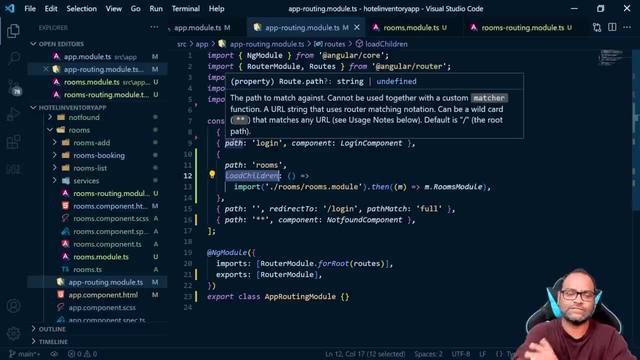 it's not like in uh. if this is a functionality which is available, we should go ahead and down. sorry, we should go ahead and implement lazy loading for all the modules. it's not lazy loading. lazy loading is useful for the modules which are really big and which you think. 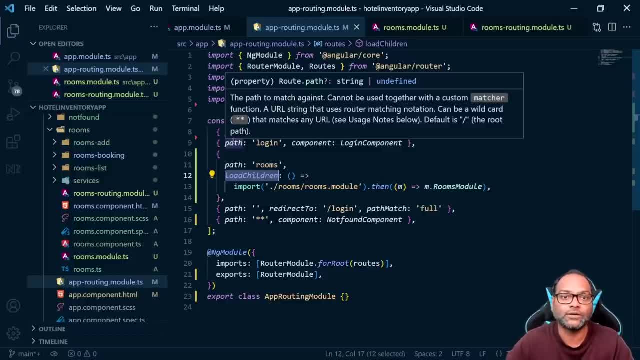 won't be used frequently by your end users, remember, not developers. developers can just go ahead and add anything, right, uh, because it's uh, it's based on the business requirement. i would say so: whenever you are implementing this, you should go ahead and ask business that okay, uh, what will be the? 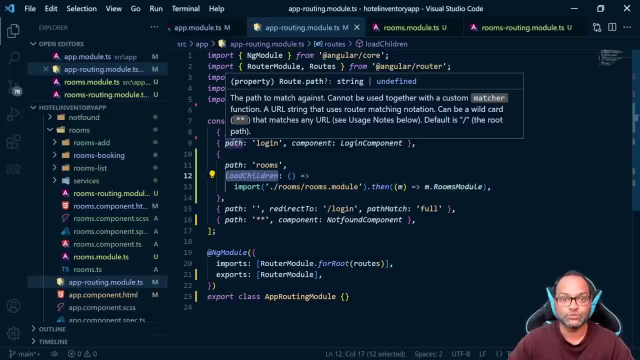 frequency how many uh users we are expecting this uh views to be used by. it's okay, in case you don't get uh. don't implement lazy loading uh at first. that's absolutely fine. i mean, it's okay uh, because you don't know your user behavior. right as you know your user behavior, you can. 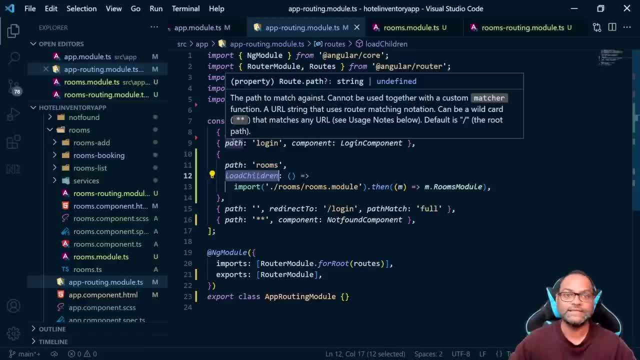 actually go ahead and implement lazy loading, but at least have feature modules in place. uh, and there will be. of course there will be many modules, which you will realize. even while developing that okay, these modules are not probably going to be used more frequently. for example, let's say you have uh user profile section. how many times you do you think uh? 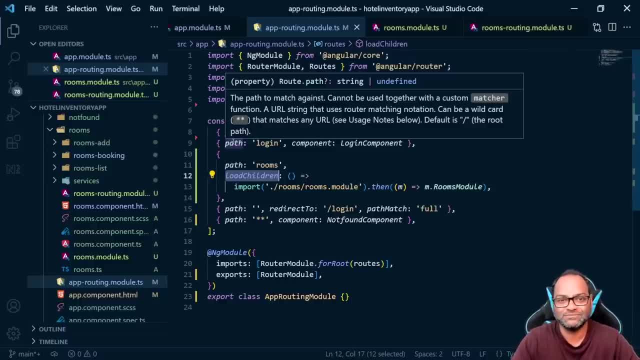 your users are actually going to use the profile section probably once in a month. that's rare, right? i mean, uh, in case they have to update some mobile number or email id, which is really rare. so those are the modules, or let's say you have some kind of reports. 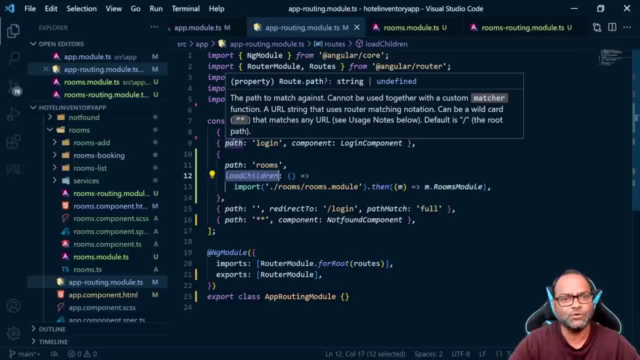 which will be, uh, let's say, which are month and report. so you know, okay, this, this reports will be, actually will be downloaded only in a month, only once in a month. so you know that, okay, this frequency will be really less. so you can go ahead and configure lazy. 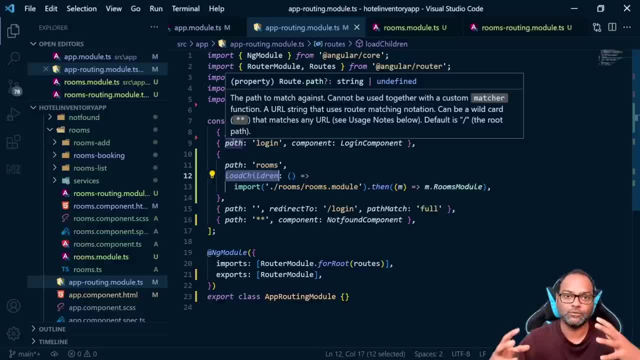 loaded module. so it's like whenever you are thinking about lazy loaded modules, it's your developer mind, as well as the business needs or the business idea which you get, how frequently it is going to be used. so keep all those things in mind before you go ahead and 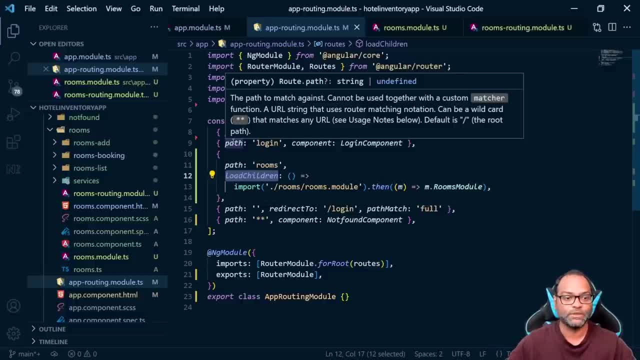 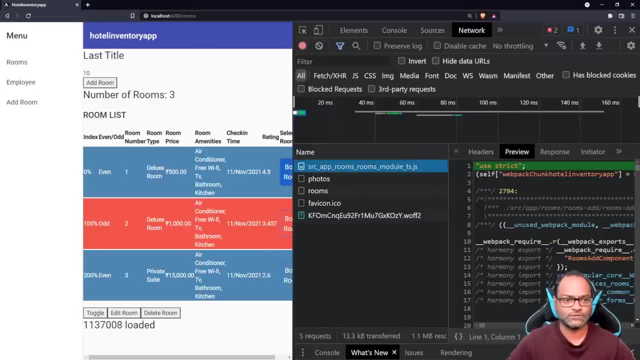 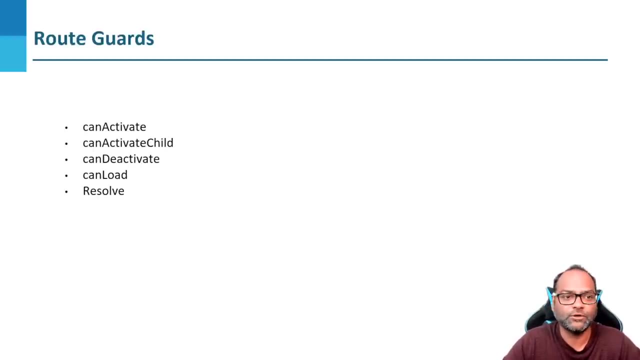 implement lazy loading, more lazy loaded module for your code base. so this is it from: lazy loaded module tried for employee. if you don't, if you're not able to do it, just let us know. now we are supposed to actually- uh, now we are going to actually discuss about ground cuttes, but we'll 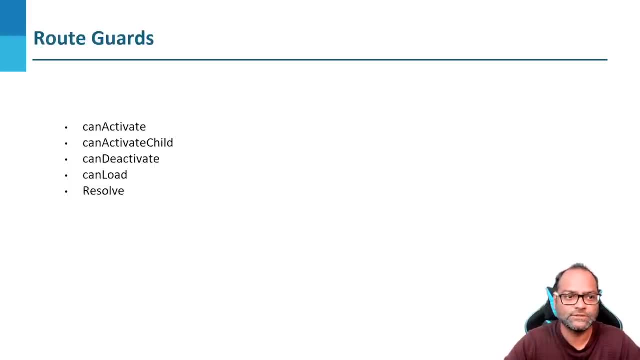 will hold this topic for few, few more things, which we will cover, and then we'll come back to the route cuts. So I'm going to show you a few more things related to the lazy loading Right now. what we have done is we already had an angular model, right we. what we did is the approach we. 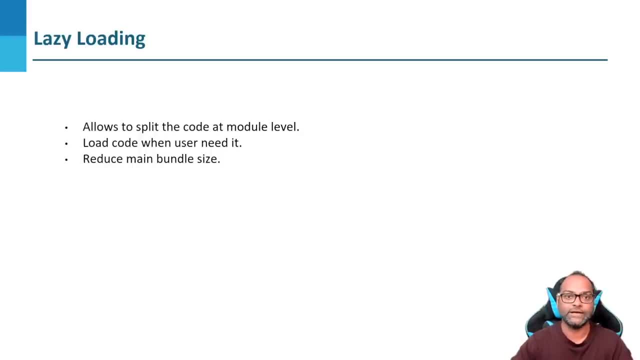 took is we created the all components, we created everything inside rooms and then we added a module, then we did a refactor and finally we ended up module which was lazy loaded. What in case, I want to start from the day when I have the requirement right. so I spoke to my business team. 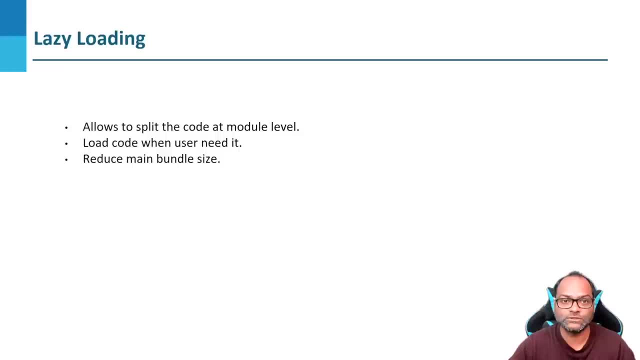 they're saying, okay, this small, this is something probably won't be used a lot, but we need this functionality. or probably this functionality is really huge and in case, if we include it in your main module, it is going to bump our bundle size. So you decide that, okay, we will lazy load it. 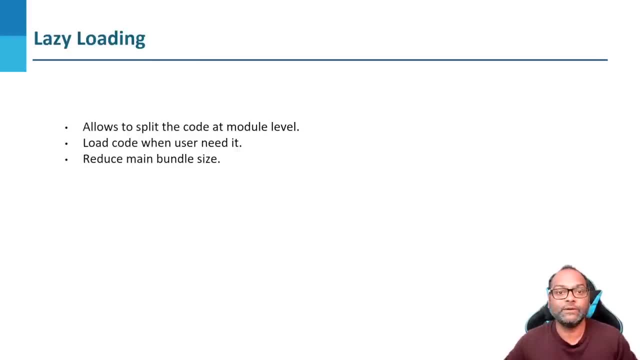 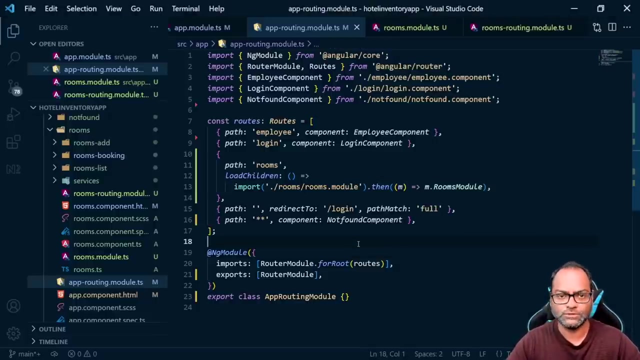 to. so the bundle size is less and it will be loaded faster for the users. and you want to start with lazy loaded module from the day one? Let's try to do that. So what we will do is we will create a module. So let's create a booking module which will show 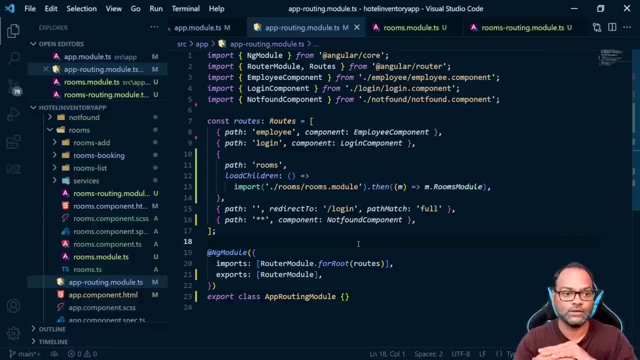 all the bookings which can be done, which will be done using the rooms module, right? So this is rooms booking, but I mean it's a great module. So this will be you used to see all the previous bookings which are made and we need to down. we need to make sure that. 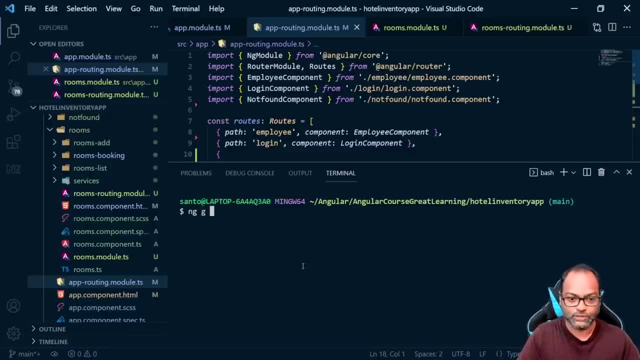 it is lazy loaded. So what you can do is there is a command to do that. So I can say ngg module. I can say a module name. so I can say booking, which is my module name. I can say hyphen- hyphen- route is equals to booking and hyphen- hyphen routing, to make sure that there is a routing module which. 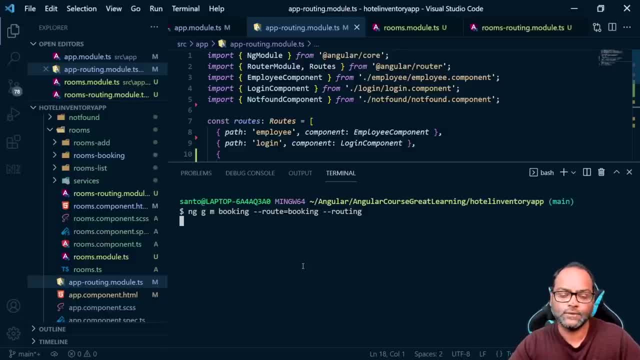 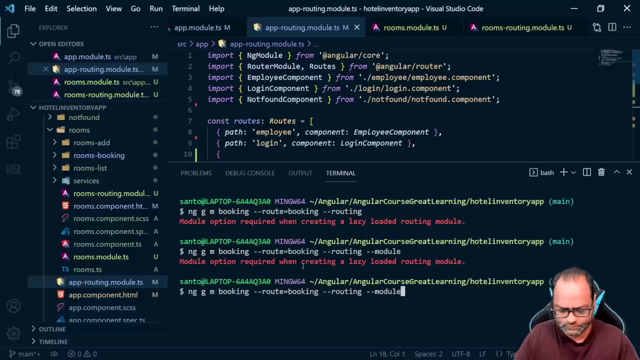 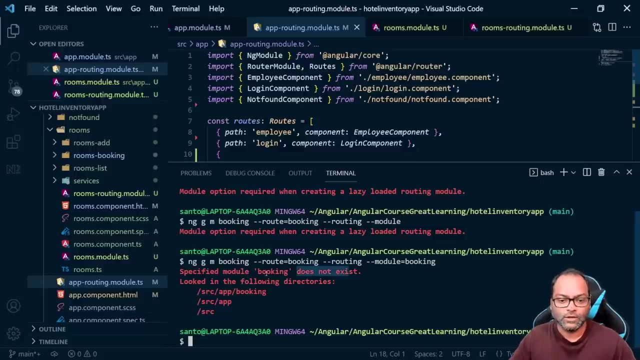 is created, So let's go ahead and enter and see what happens. module option required. module option required: when I can have an module is equals to booking. Let's see our, I think let's see Song p lawn: p neues, p p новый. 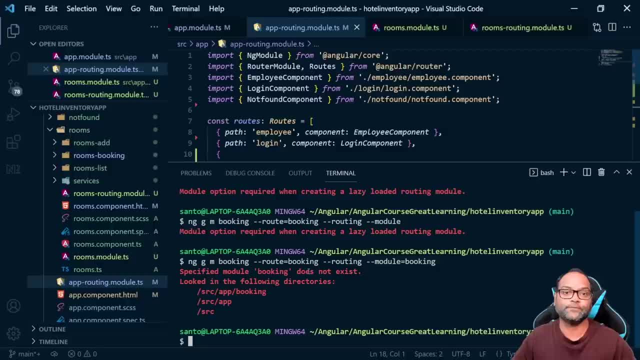 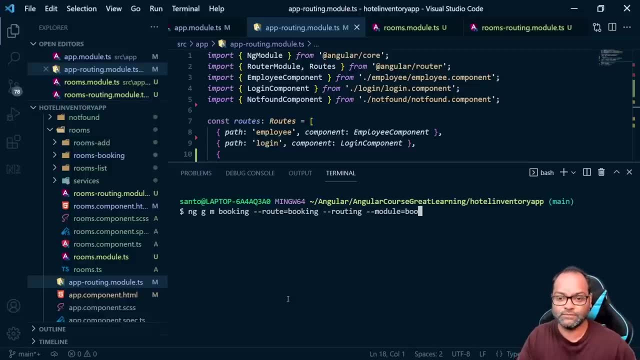 songs. module booking in the next class, modulecom. So let us do this. here is so: modulo does not exist. Okay, So there was a problem with the command. Now let me just talk about this particular module, So what this module is. so it is asking me, where should I go ahead? and 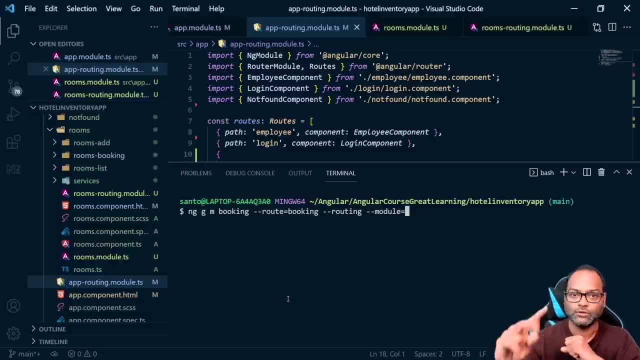 register this particular lazy loaded module. Right now we have two modules: rooms module as well as app module. So we have to provide the module where we need to go ahead and create a lazy loaded route like this. So right now, what I need is: I want to create it with app, with app module. 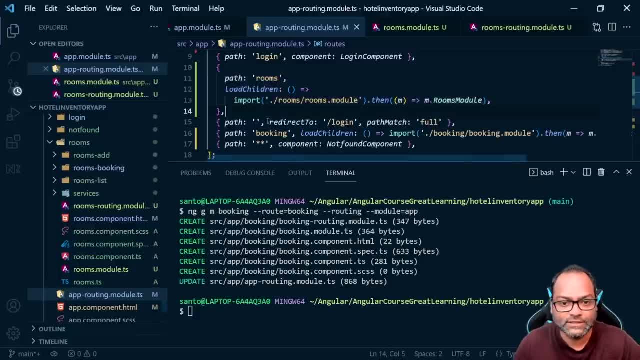 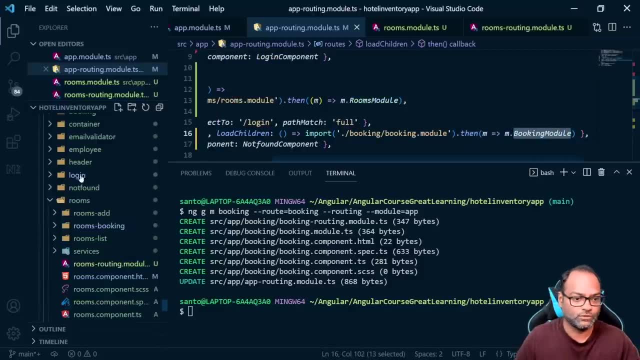 So it will now go ahead and create- you can see it created a path here. So you can see: booking load, children import booking module and booking module. So if I go to booking module now, you will find several things. You will find a module, you will find a component and all the 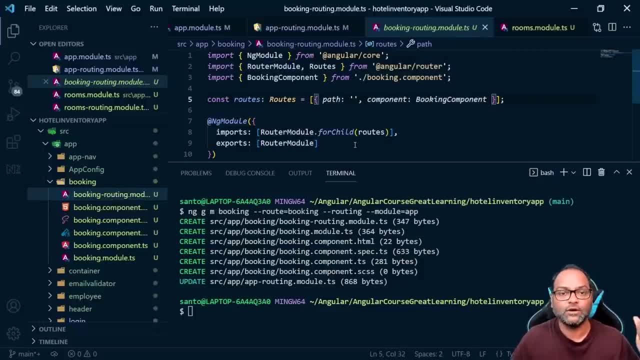 related files, as well as booking routing module as well. All this by using a single command, So you don't have to go ahead and do whatever we did earlier, right? So go ahead and create component and add a module and then do this. No, you can just do it with a single command. Also, I'll show one more command. 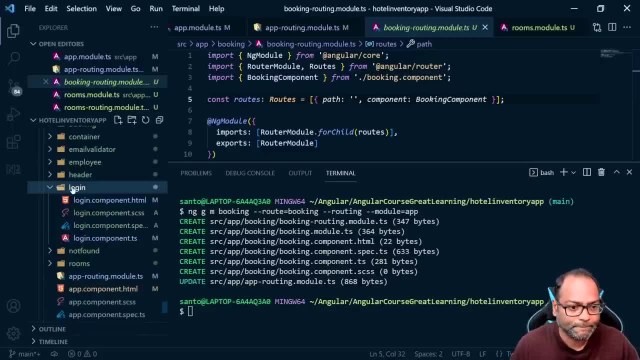 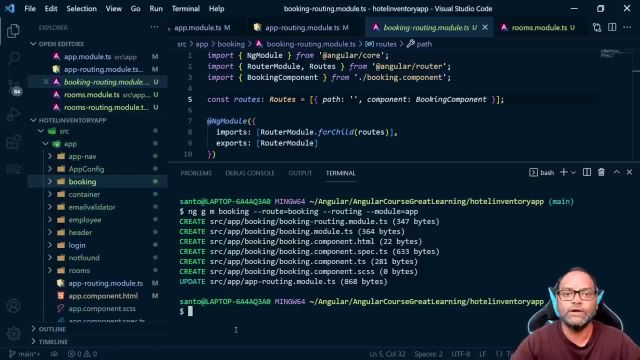 which we can use. So, let's say, is there any other screen we want to create? Okay, So let's say, I want to create a filter functionality, right, So where we can search for, like search functionality. So we we want to search for rooms and we what? 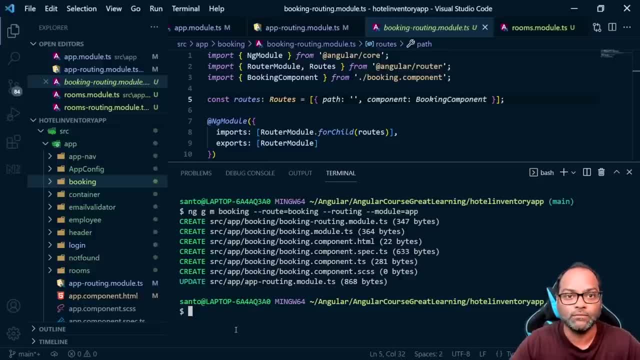 we want to do is we want to create a module first and then we want to add components, and we don't want to lazy load this. Remember this one? we wanted to lazy load this one and we don't want to lazy load. So what we can do is we can create first the module, So I can say NGG M and I can say 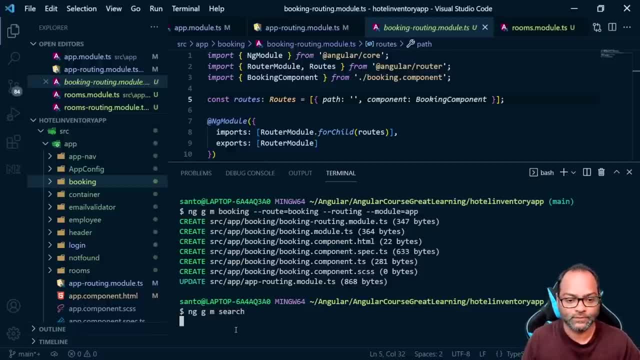 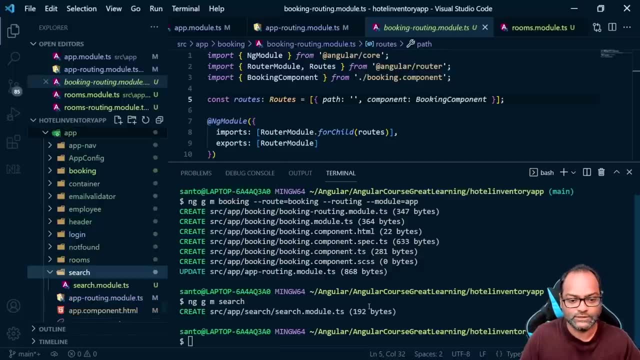 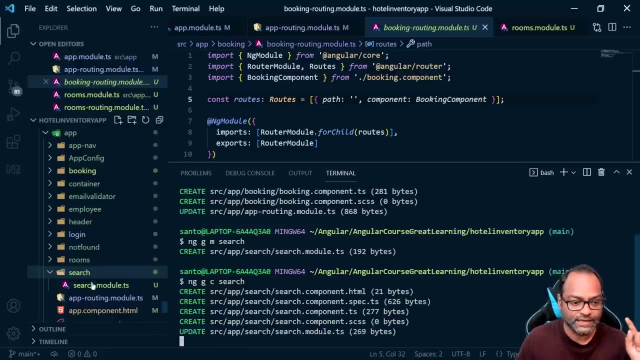 search. So it will create a module first, right. So now we have the module. Now I want to create a component. So what I can do is I can just go ahead and say NGG C Search. Now this will create a search component inside the search folder. So you can see. 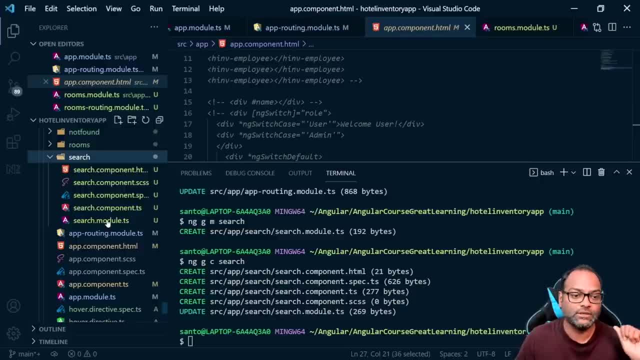 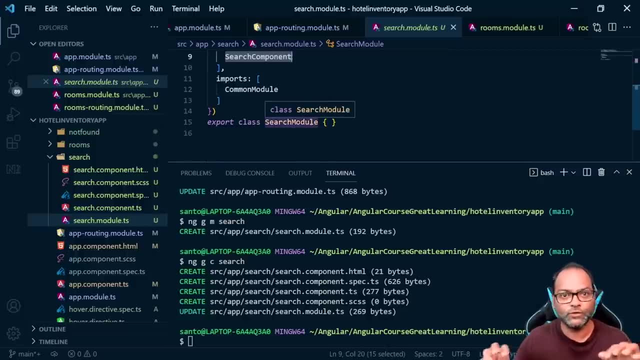 it created the files inside search folder, as well as one more thing: search module will register this search component. So this is all all done automatically. You don't have to do it manually. The only reason I went through, or I went through the 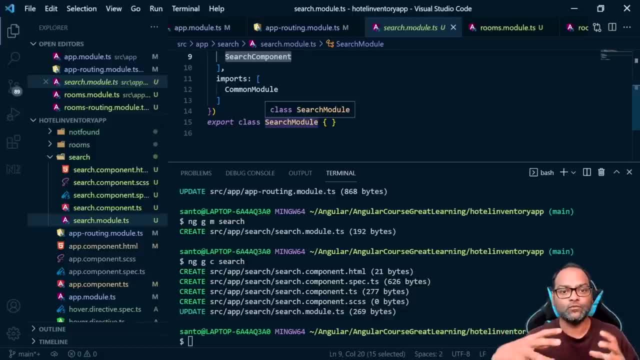 the path where I did everything manually is probably you won't be writing the code from the scratch in your application. You should know how to refactor the application or how to revisit the code, right? I mean what's wrong, what's right in your code base. 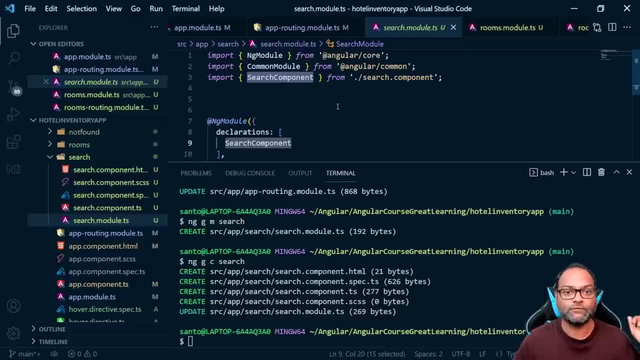 Otherwise you will be lost. So that was the whole purpose of actually doing that exercise. In case you are creating new code, this is the way you should be doing it, So first create the module and then create the component, in case it needs to be lazy, loaded from. 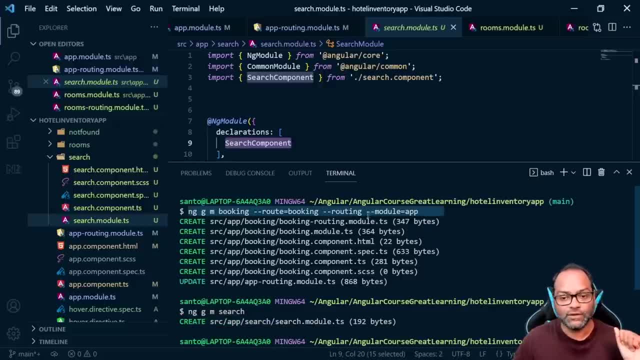 the day one. just go ahead and reuse this command and that's it, And you can define which on which module I want to actually register it. So you can define which module I want to actually register it. I could have given it as rooms as well, Remember this, So in case I'm going to actually access this, 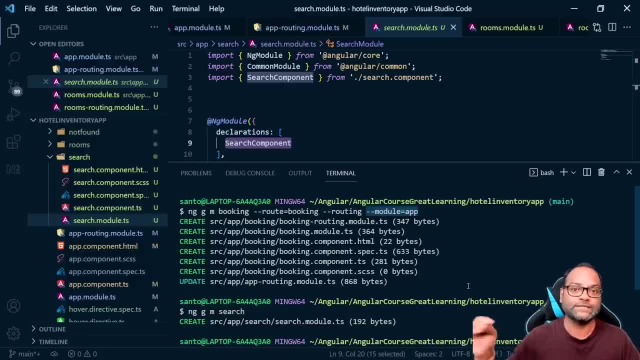 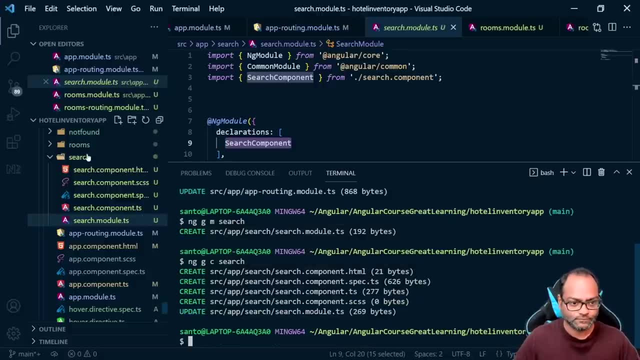 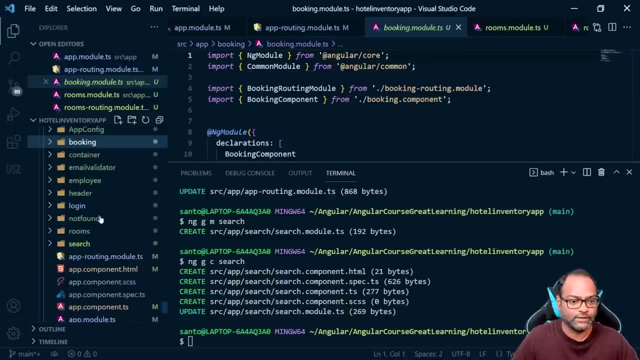 from the rooms module. I can do that, So I can actually lazy load any other module inside rooms. That's also possible, Probably we'll try one exercise with that as well. Now we have our booking module and this is lazy loaded as well. So now I can just go ahead and add navigation and 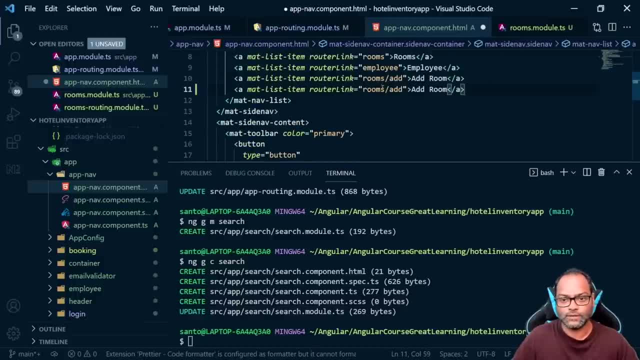 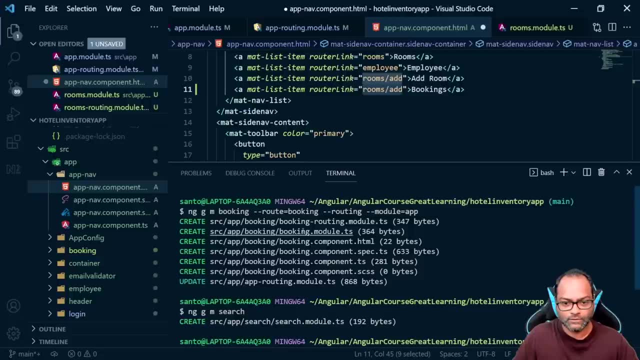 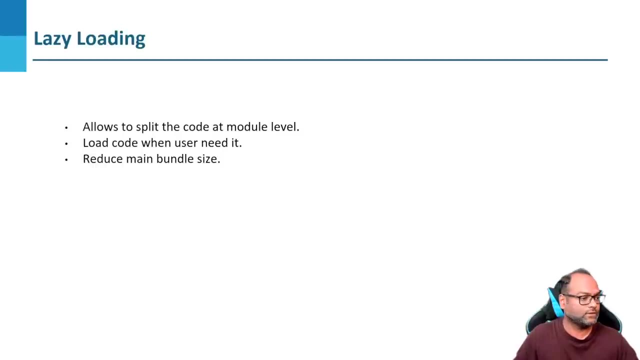 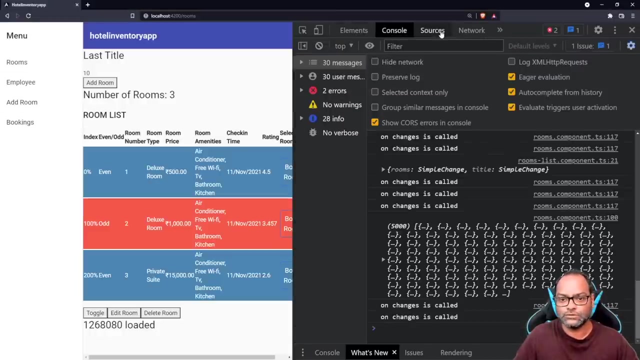 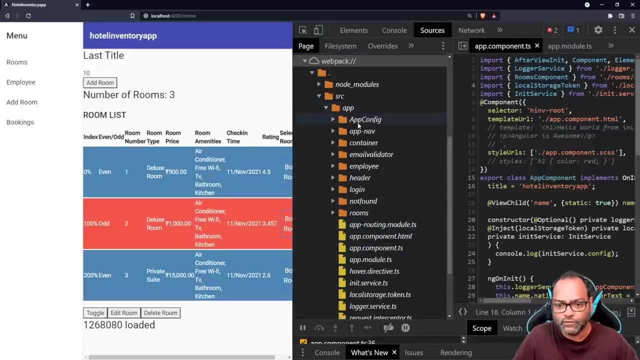 we can say: this is bookings, and what was the route booking? and let's revisit the application. and you, uh, let's go to sources, the pack dot slash SRC app, And you can see we don't have anything related to booking. Let's click on bookings. 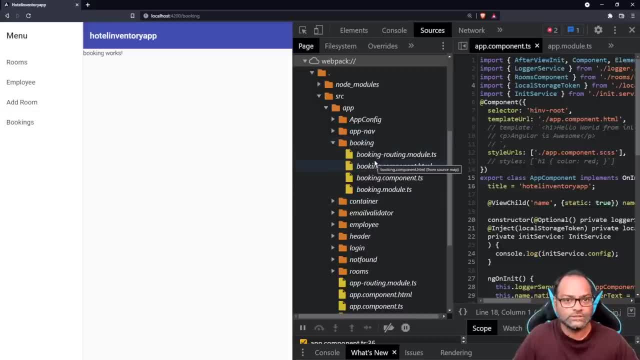 And now you have everything related to booking. So this is another command, another way to do it, And we will, of course, go ahead and add a form where we can see all the bookings in in upcoming videos. right, So we will be using angular material table. We'll show you an example. 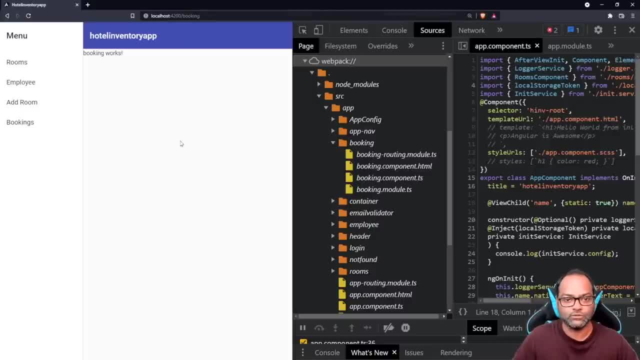 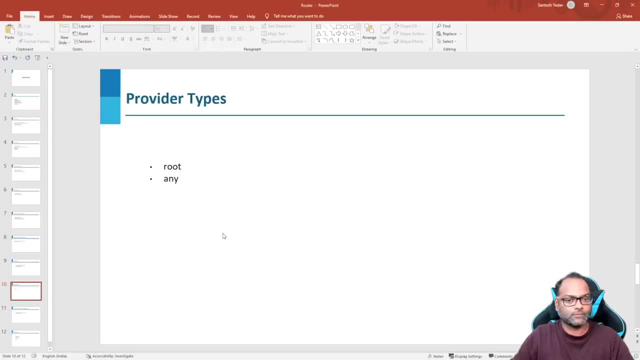 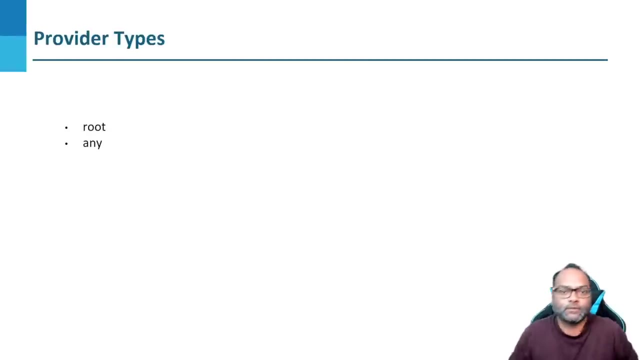 of how you can utilize angular material table to do that. So yeah, that's another way to implement lazy loading. So when discussing dependency injection, if you remember, we left one thing. I mean, we said we will be discussing about it once we go through the lazy loading. So let's go back and do. 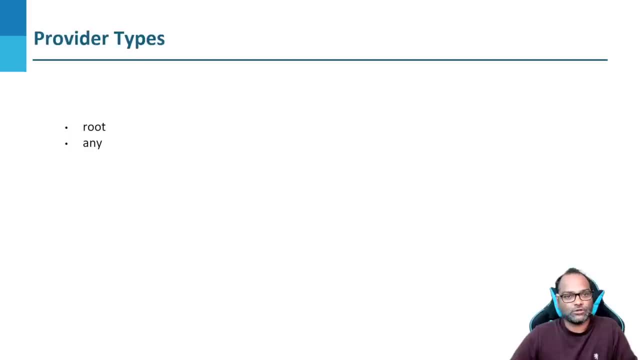 that. So we discussed about provider types. We saw a route right. We said: okay, in case it is route, you can actually go ahead and add a use: this particular- uh sorry, you can use that particular service as a singleton service across your application. Now we will talk about the other. 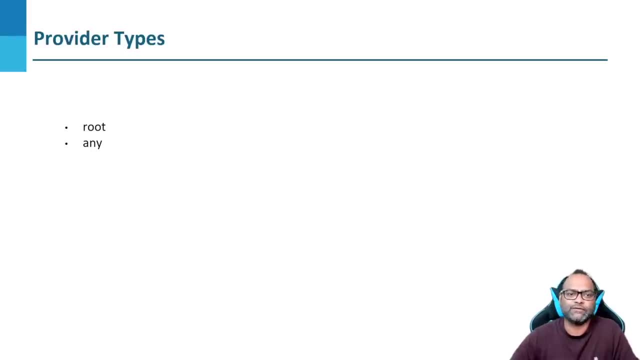 type of provider type, which is any. Now you might be wondering where this Inie is useful, So let's go ahead and talk a little bit about it. There are there are multiple use cases, and I wrote a blog post on the same, So I'll be trying to cover the same example here. 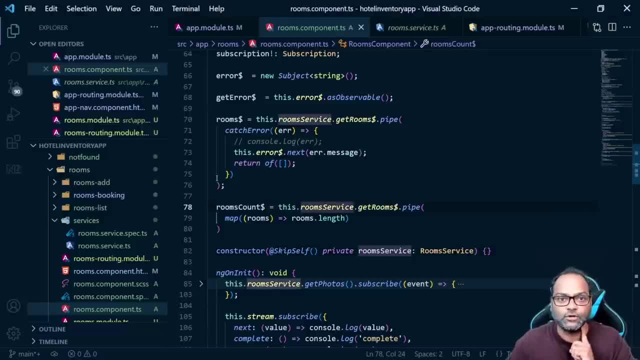 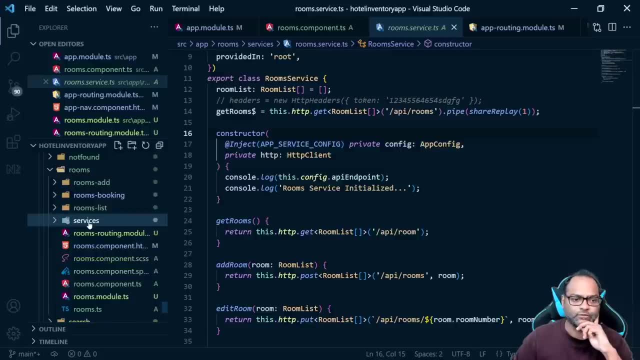 but let's figure out what is the use case for using any. so here let's say: we have a service like we. uh, what we will do is: we'll create a service, we will call it as a config service. we already have app config, so let's create another service and for that i'll be creating a services folder. 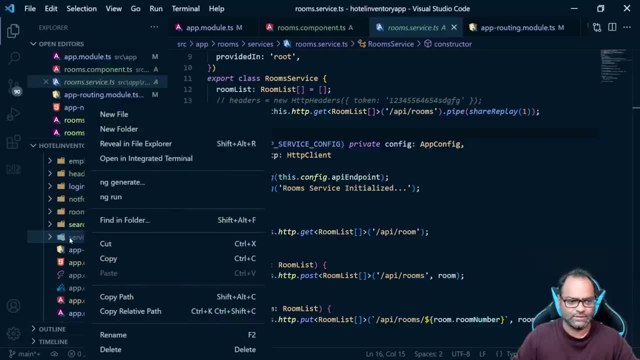 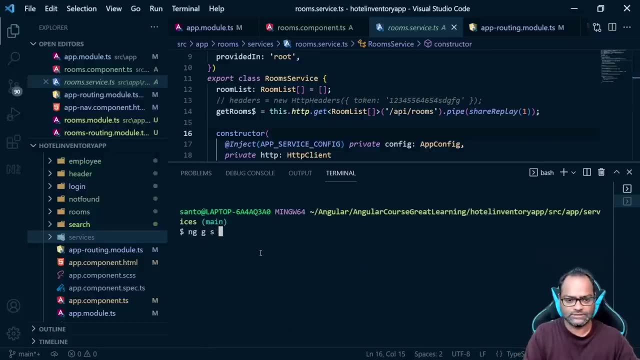 so this is like a reusable kind of services and let's and open the integrated terminal. i'll say nggs and i'll say this is uh, what should we name it config? let's call it as config service. i don't, i don't think so we have anything. 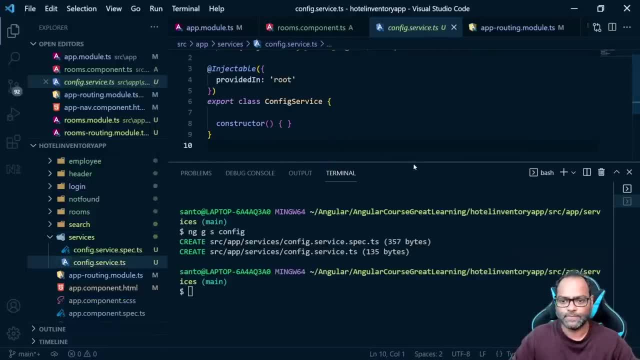 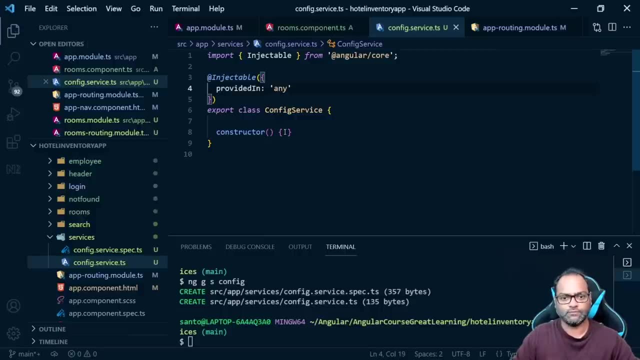 called config service as of now and here. so we have this config service. let's go ahead and change this to any, and one thing which we will be doing is we will be, uh, let's do uh, console dot log and let's see how many instances get gets created. so we know that. 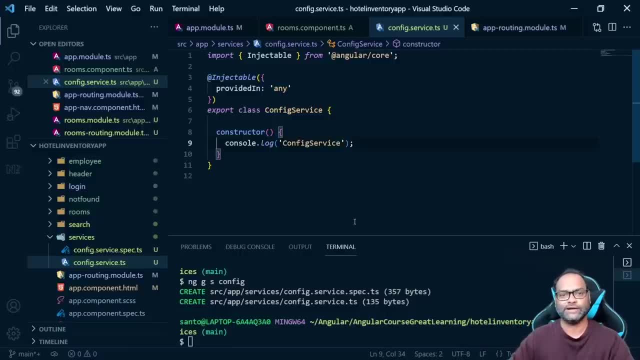 whenever a service is configured with provided in root, we get a singleton instance and we, in case you want to create multiple instances, you can just go ahead and use providers property, as we saw earlier now, using provided in any. let's see, uh, what happens. so i'm going to use this. 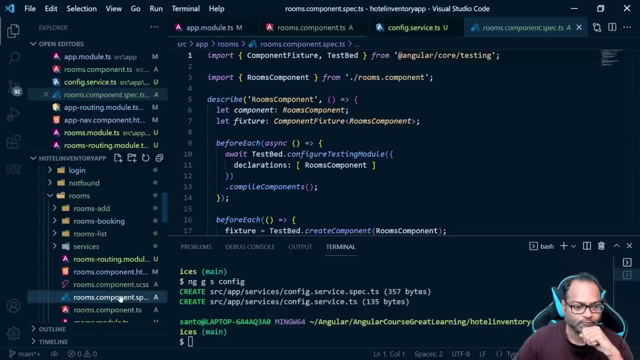 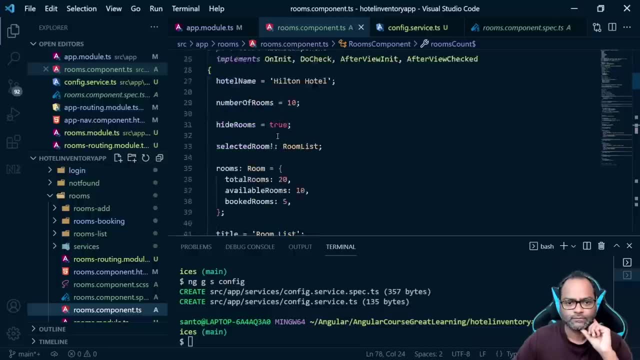 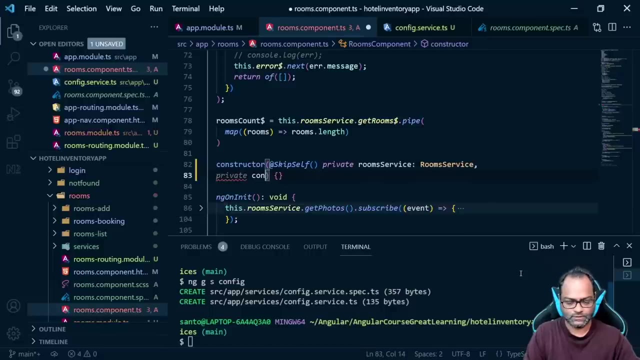 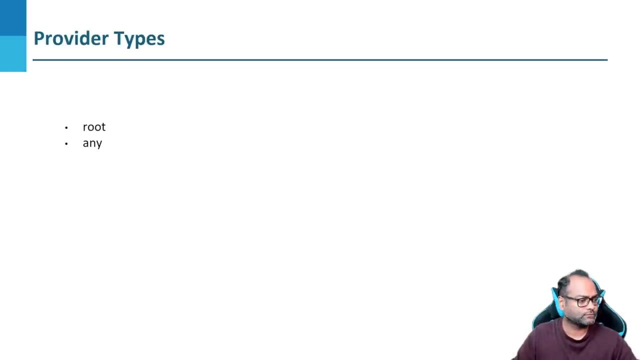 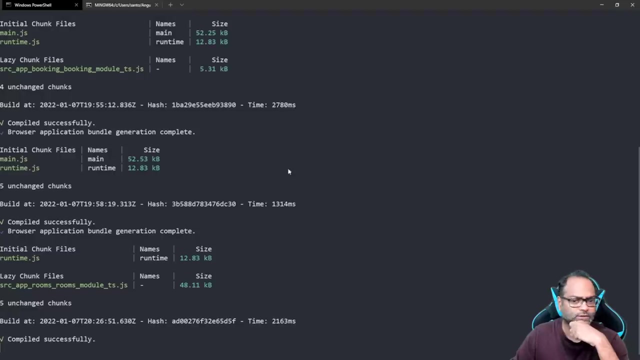 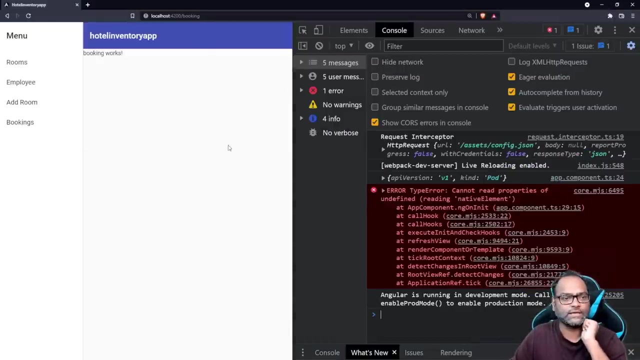 service inside the rooms component. we'll just inject it as of now. let's say this is private config service, which is type of config service, and let's go back to the application. let's see: uh, it is compiled. yeah, now let's go to console, and this is where we will. we want to see an interesting thing, so here let's use config services at one. 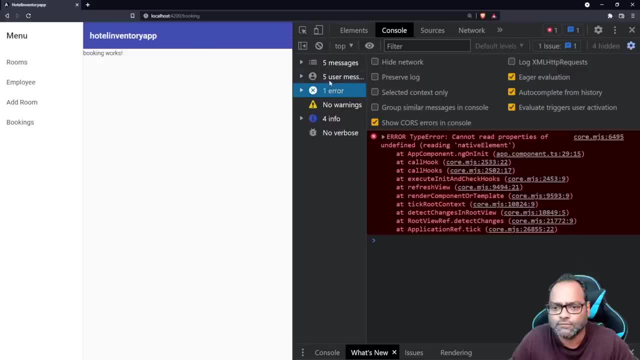 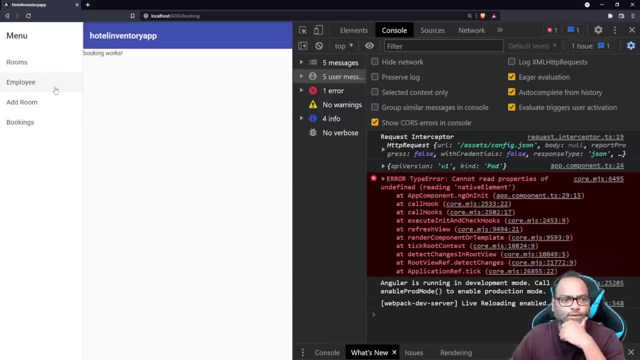 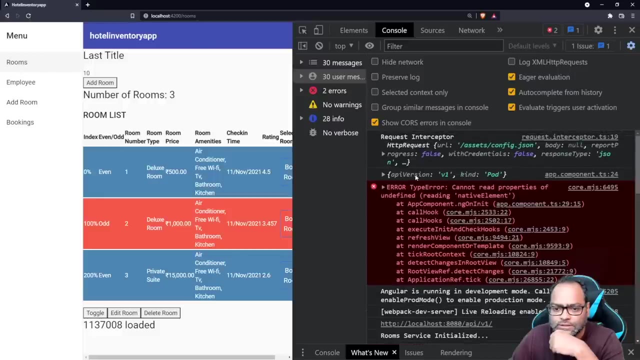 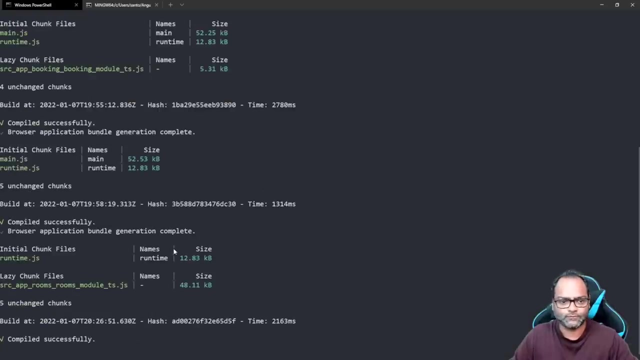 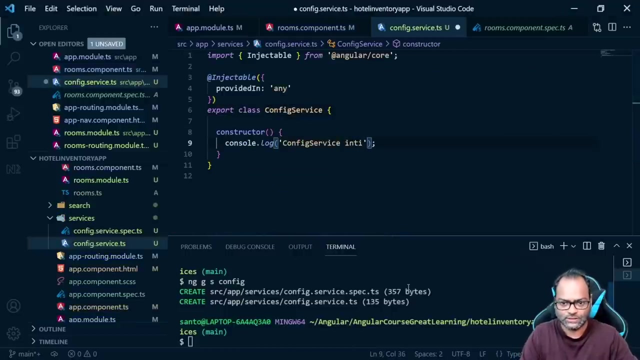 place other, or is it okay? Okay, let's do control F5, let's click on rooms and here I'll see. let's see if we have this room service initialized, config service, right. So config service initialized and we will be using the same config service inside app. 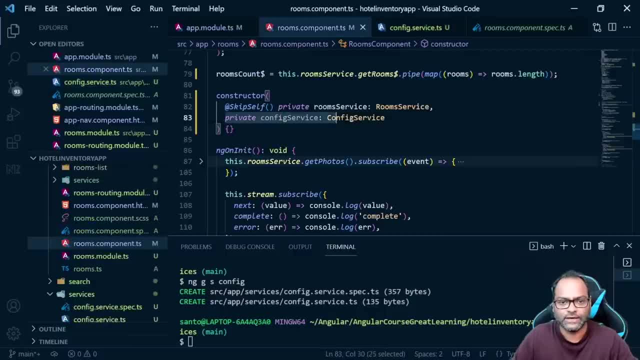 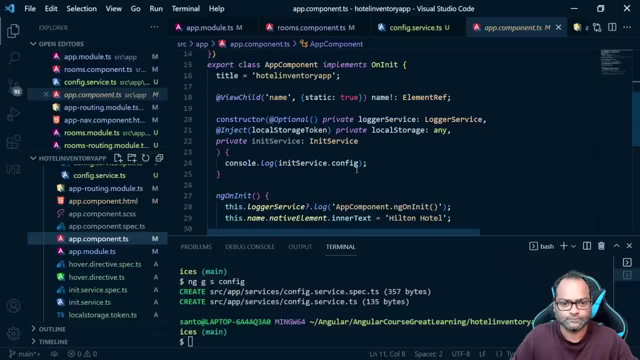 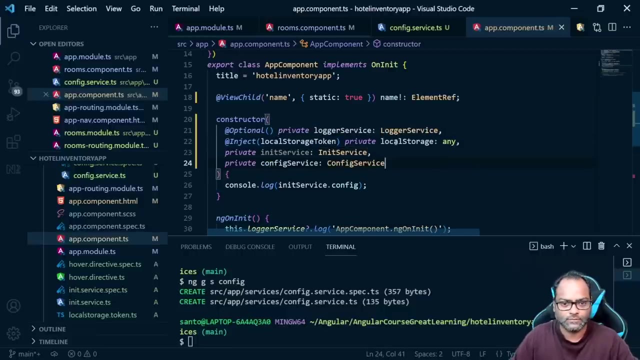 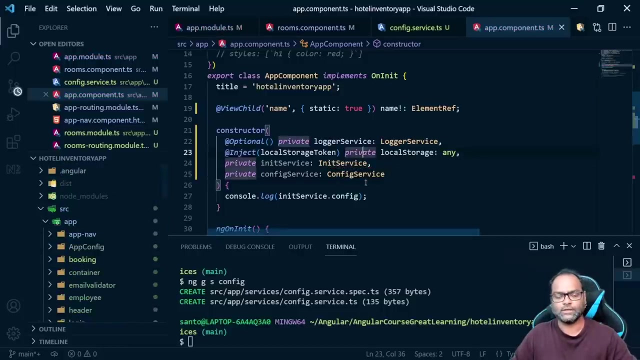 component the same way. I mean, we are not going to use it, We'll just inject it and see how it behaves. Constructor- this is the constructor And let's see if we have any other module. that's okay. again, those two modules are: 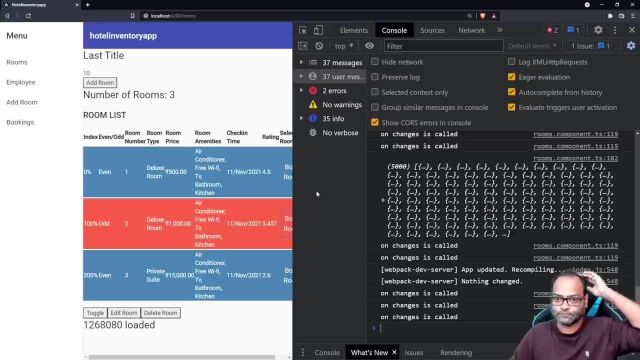 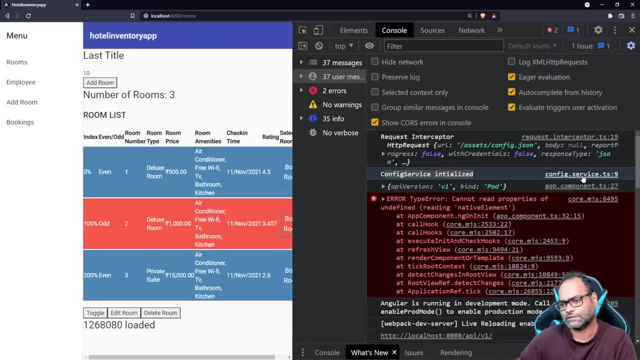 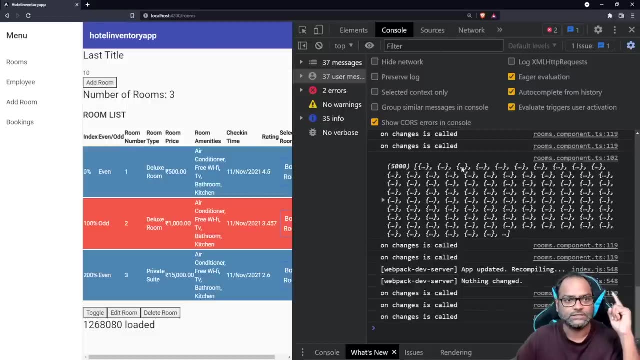 enough, more than enough. Let's go back to the UI. and now you can see: uh, here it says config service initialized. So we have config service dot TS, line number nine. It means one instance of config service is created right now and we cannot see any other. 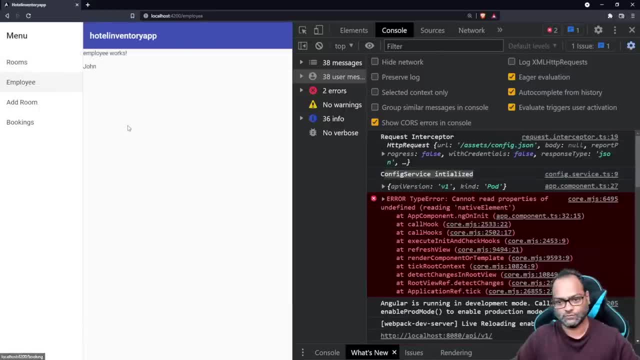 instances which are available. Ah, okay, To do one more thing, I'll just clear this and let's see the messages. So we have this config service initialized. So now, why actually, uh, moved away from rooms? Because on click of rooms, I mean it- it is supposed to create another instance. 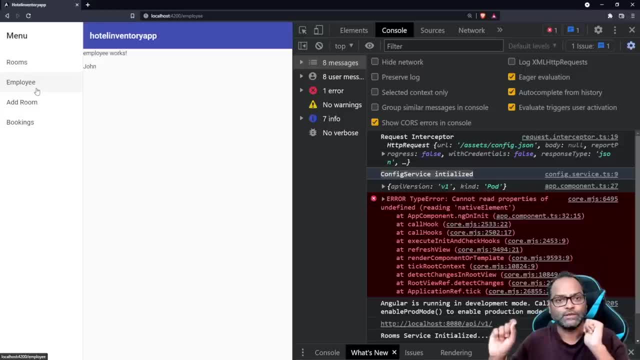 So let me tell you why we have not done providers property. We have not added a provider's property. Why shouldn't it create a new instance? So let's go back, go go ahead and talk about how any plays an important role here. 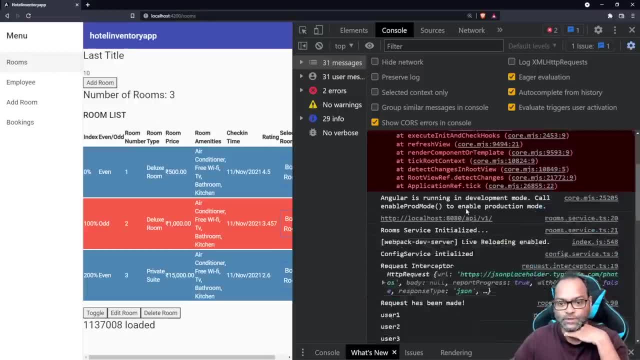 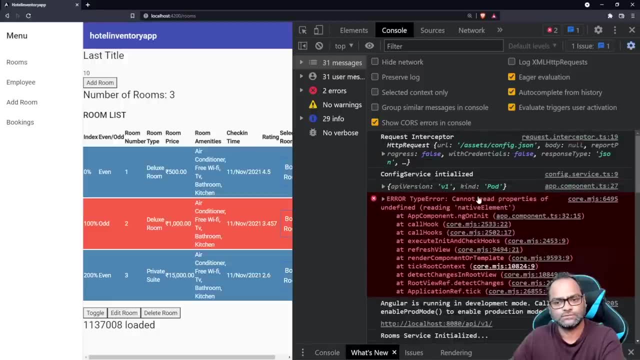 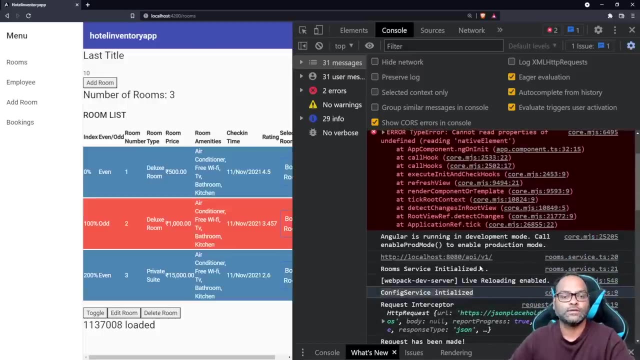 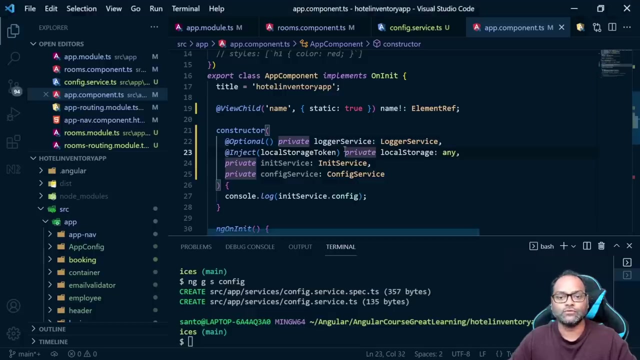 So we have config service initialized here. Let's go ahead and click on rooms and you will find that here config service is initialized again. One instance, two instance: why so? So when we say con this providers, sorry, so when we use this providers at provider, 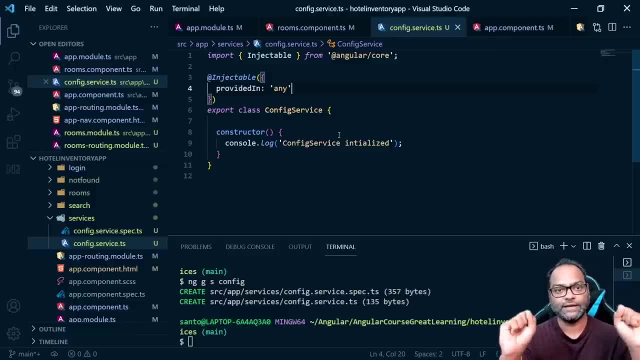 in as any. Okay, It will create one instance for the entire code base where there's nothing lazy loaded right, And it will create separate instances for each lazy loaded module in case it is getting used. For example, it is getting used in rooms. 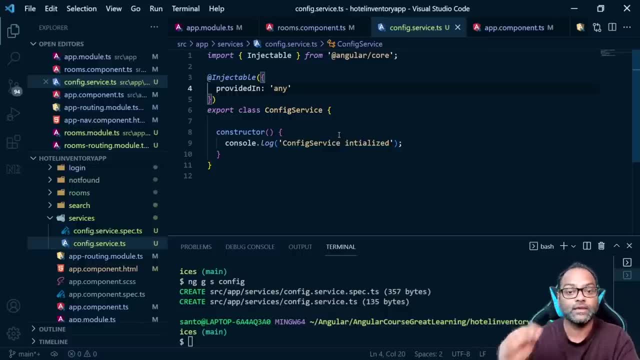 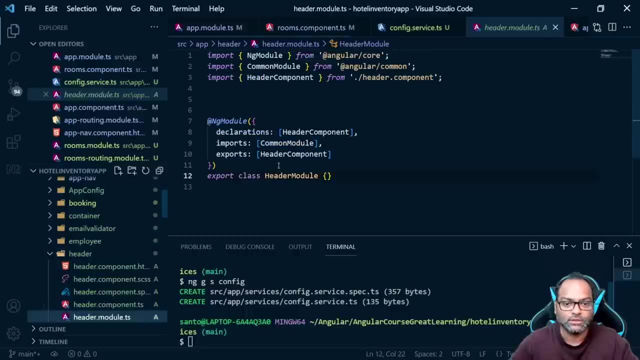 So it will create another instance for rooms module. If we go ahead and inject it inside, let's say: um, we have another model called header. Okay, If we inject another instance in header, it will not create another instance because it is not lazy loaded. but let's go ahead and inject, let's try to inject it and see right. 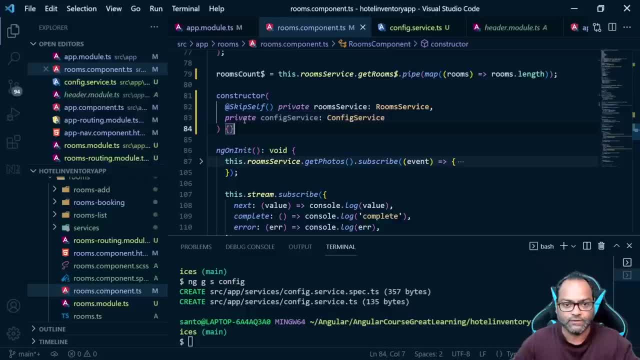 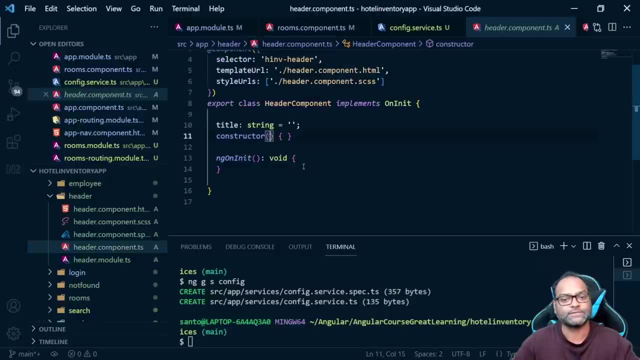 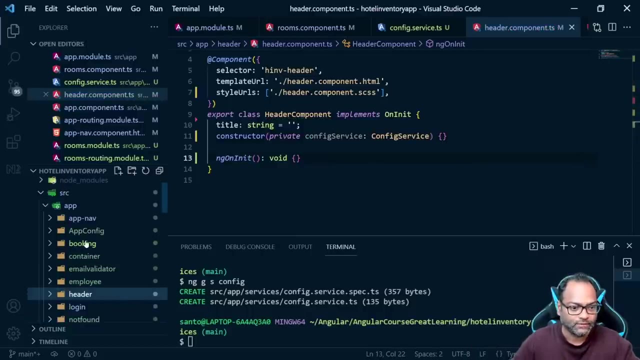 So how many instances we end up with. So here, uh, we have copy this header So as, as per expectation, header uh should use the global instance which is available, which will be created, and we'll create one for booking, because booking is lazy, loaded. 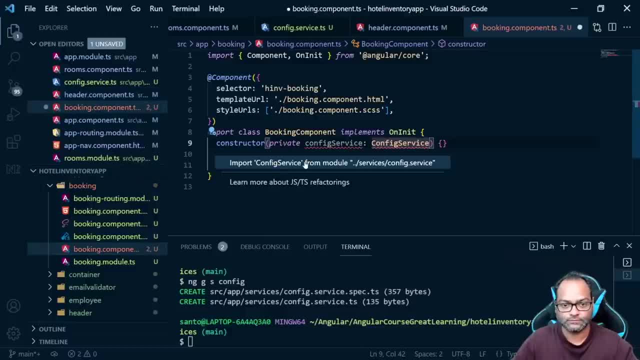 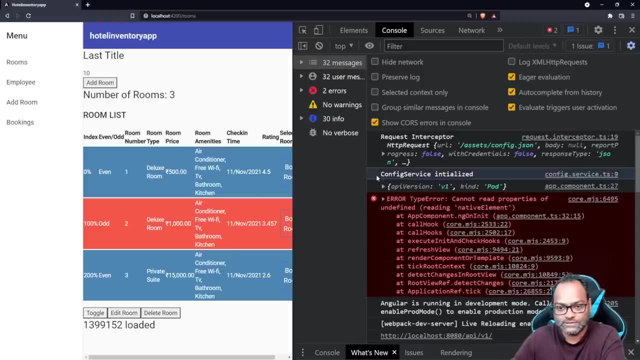 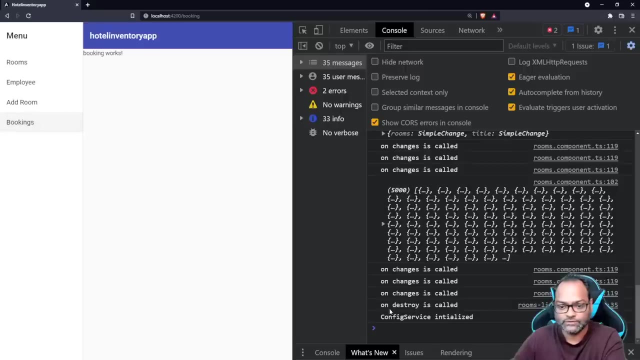 So let's see now rooms has a, so one is global instance config service initialize. then rooms has another instance config service, initialize two. And now let's click on bookings. And once we click on bookings, booking has another config service initialize. 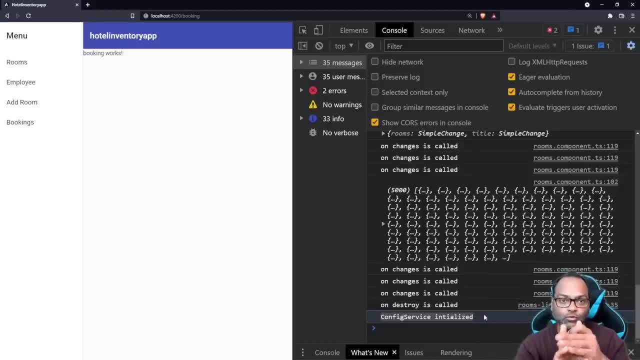 So we have how many instances right now, three instances- to use two separate instances used by two different lazy loaded modules. As we said, two separate instances, Provided is any and when, which is global instance, which is available everywhere. What can be the good use case? 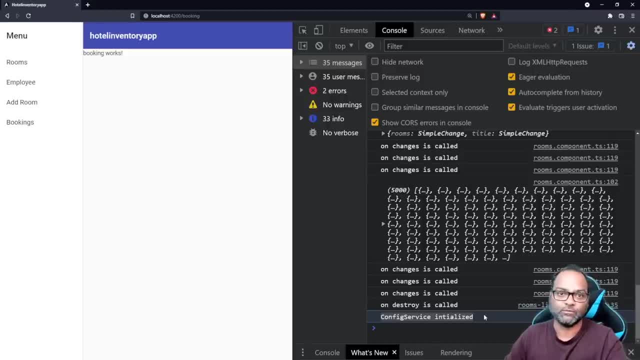 So let me just give you an interesting use case which actually wrote a blog post on and it is great It is actually used in um one of my friend's book which was launched. Let me just talk Uh so uh, which was launched last year. 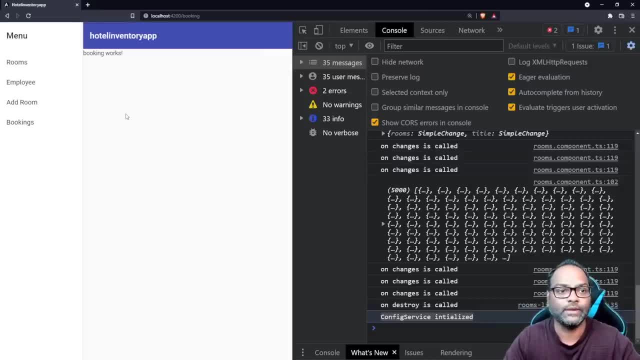 Yeah, it was launched last year. Uh, it is a big book based on angular Ivy, So it's it's a little bit advanced right now. you are on basics. So I'll say I suggest, once you have the basic idea or a little bit idea about angular, how it works. 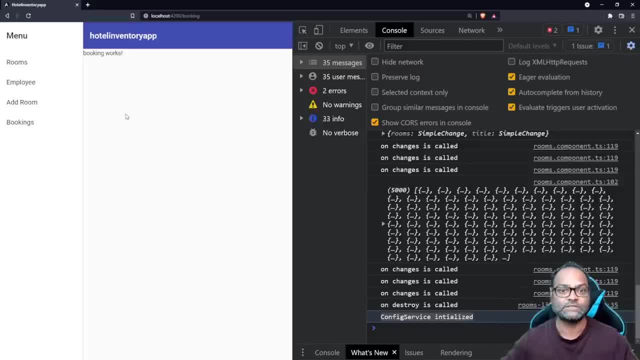 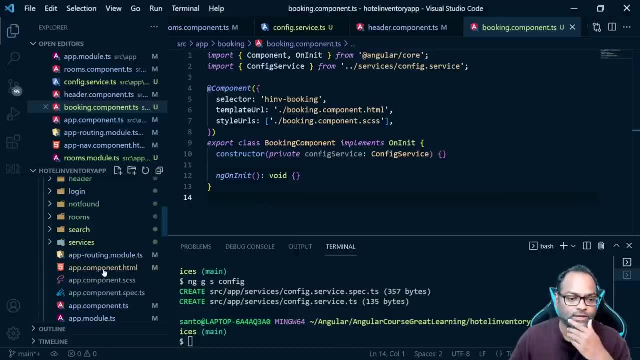 then just go ahead and purchase that book. So it's on angular Ivy, which I actually proffered. So let's go ahead and talk about the use case which I was talking about. So here, what we will do is I'll create another. uh, so we already have service and I will. 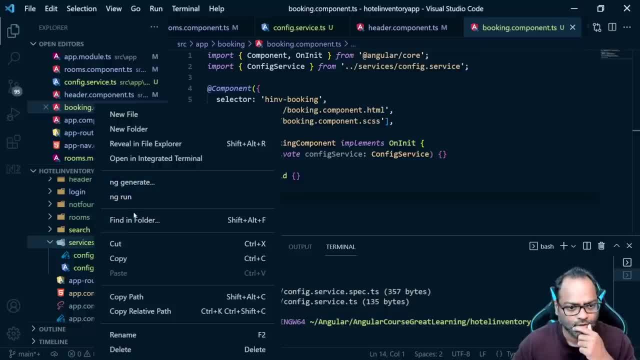 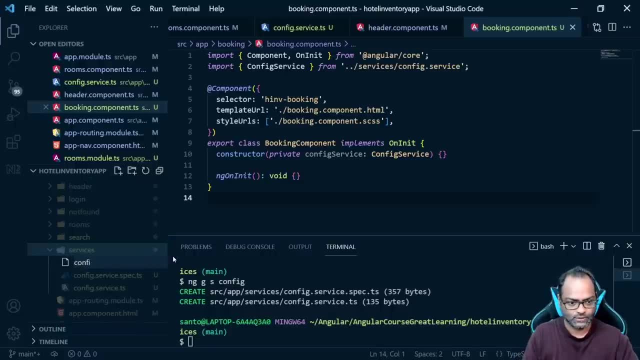 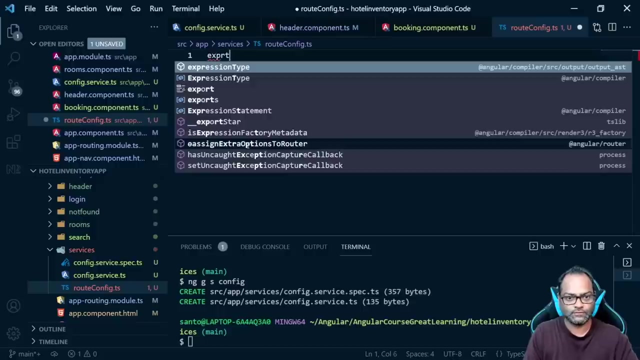 create one Injection token And say this is a: Okay, Okay, Sorry about that, Let's go ahead and we'll call it um config, Let's call it as route config. So this interface, uh, this would be the interface, and we'll say this as export interface out. 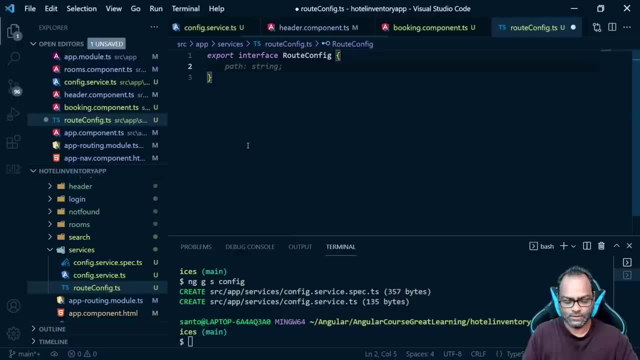 config, Okay, And we'll say: this is uh type of service, We'll give it a name. Well, I'll just give it a name type of string. so we have just single property. and let's create an injection token. so i'll say: 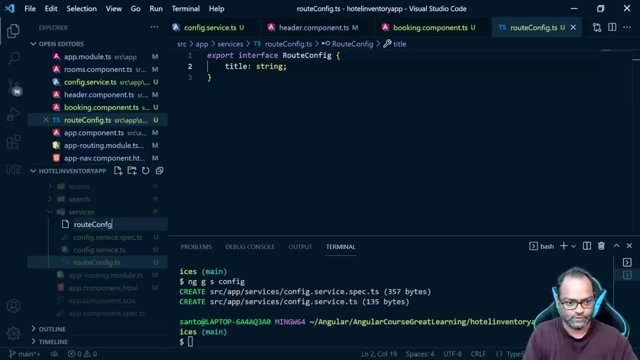 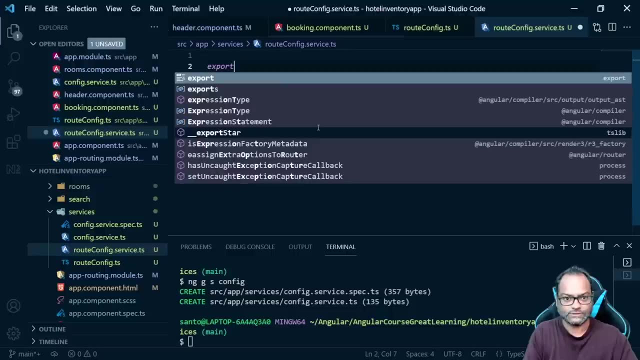 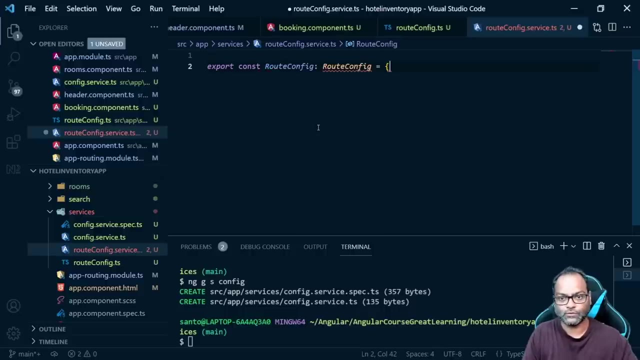 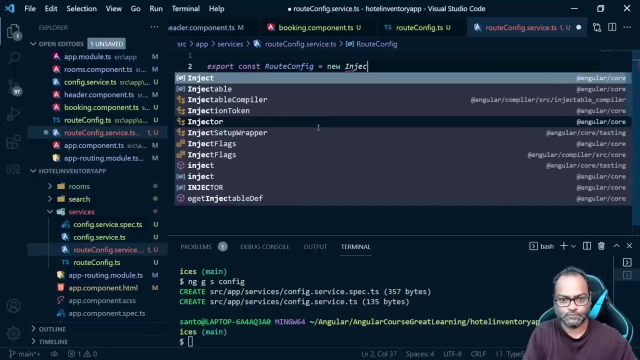 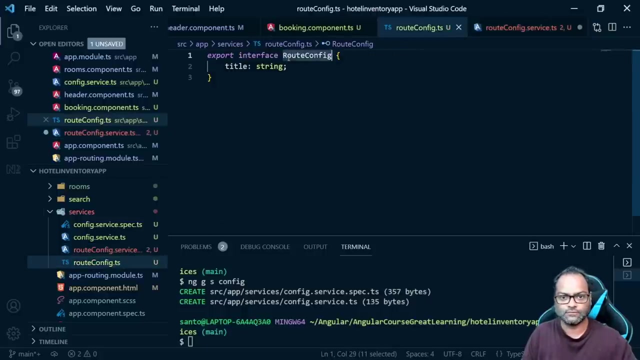 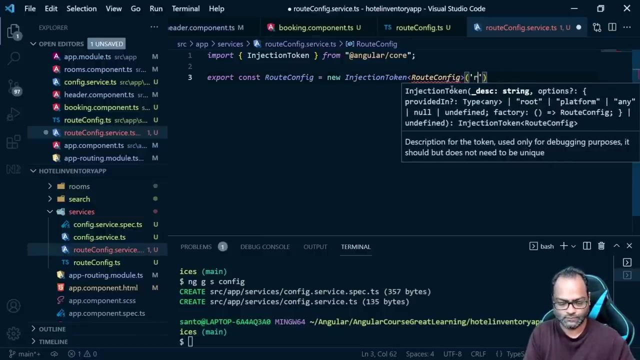 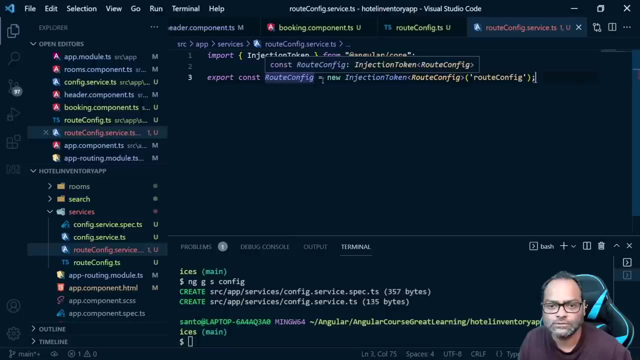 this is route config, dot, service, dot, ps. and here we'll say export const route config, which is equals to new injection token, which will be type of this particular interface. and i'll say: this is a route config. and what is this route config device to? where it's being used as a type? 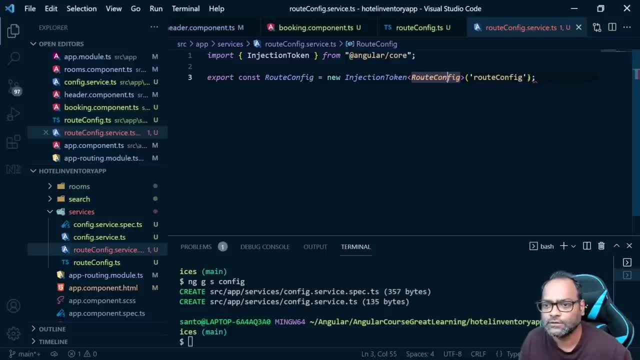 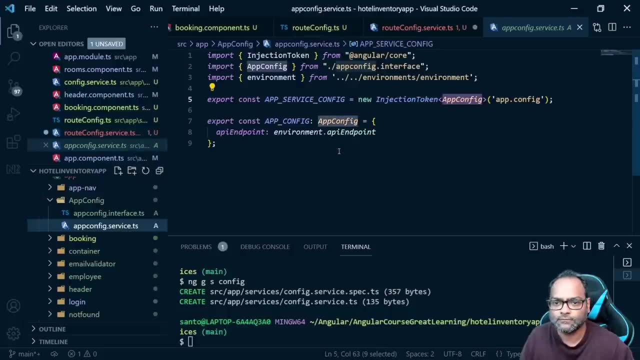 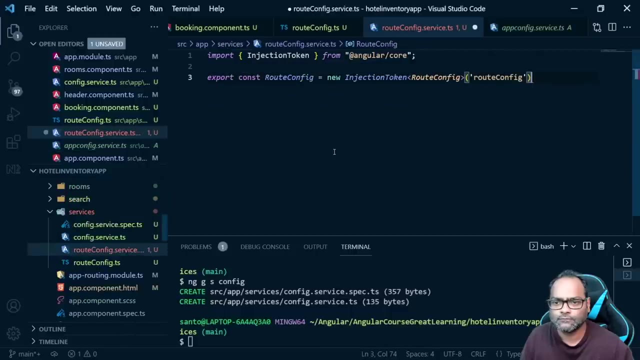 name injection token, which is type of route config. okay, let's see what i'm missing here. ah, this route config which is looks like this is something which already exists in angular core and let's import this, import the interface dot slash route config and we'll say: this is the interface which we are looking at and 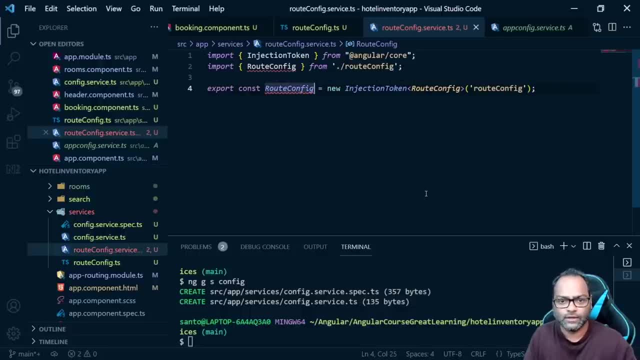 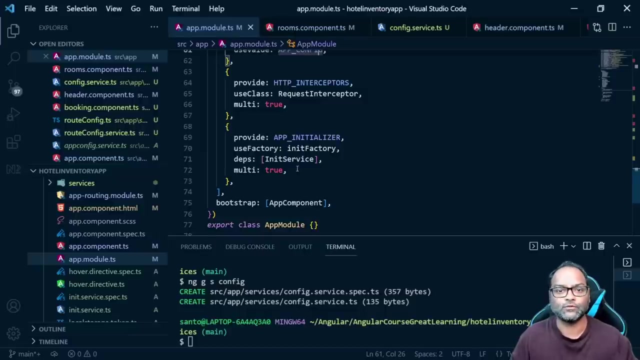 This should be fine. route-config-token- great. So we created our token and now we have an interface. Let's see how actually it helps in case we are using. provided in as any, I'll use this route-config-token in AppModule. we know how to do that right. 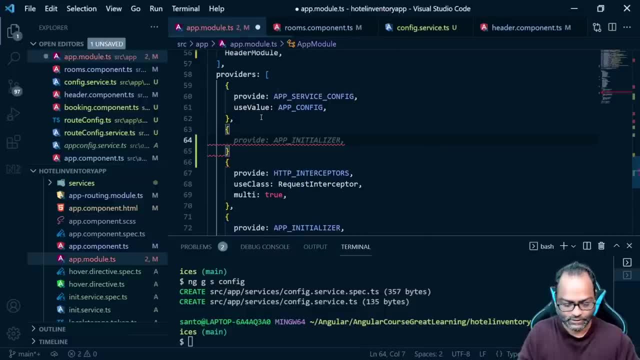 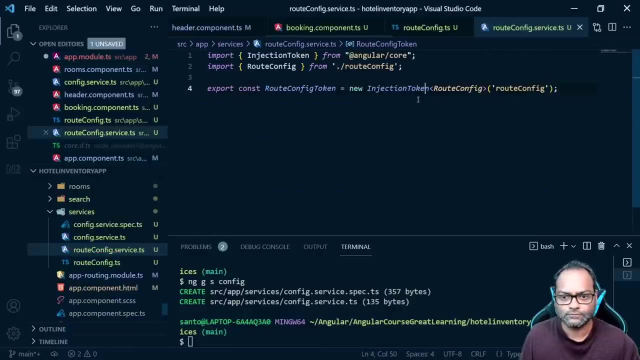 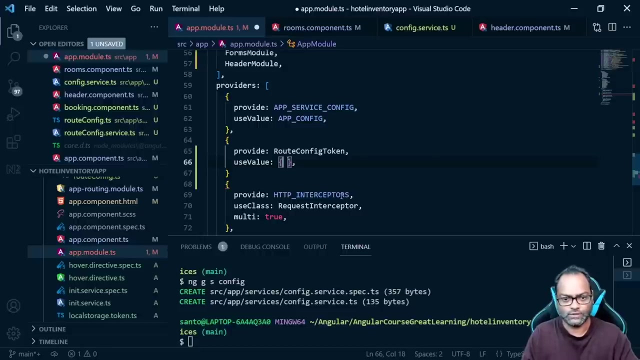 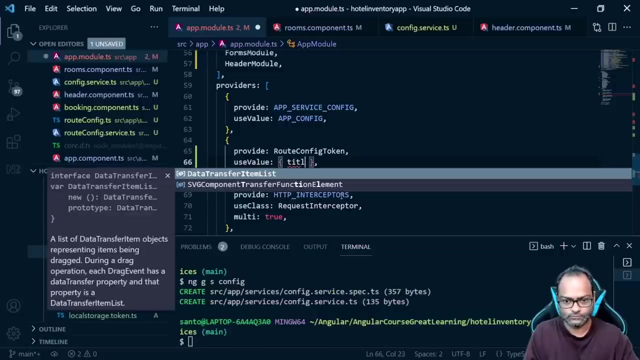 So we already have an example here. So I'll just add provide and we'll use value, which will be: Let's go back to AppModule and we'll say which we'll be having. So we know the type. So we have this title, which is home. 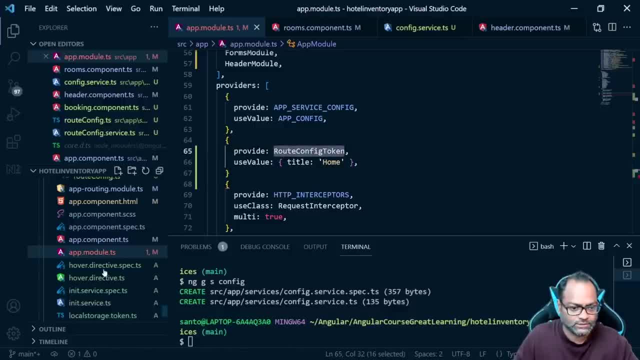 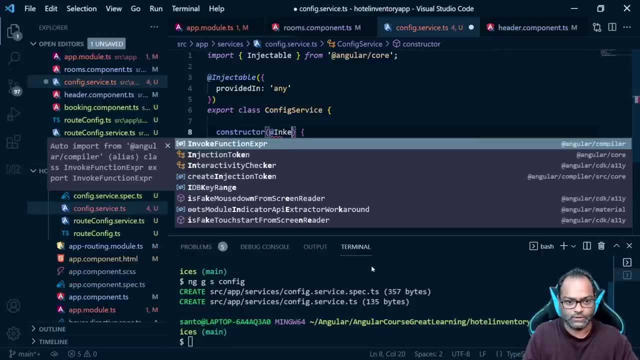 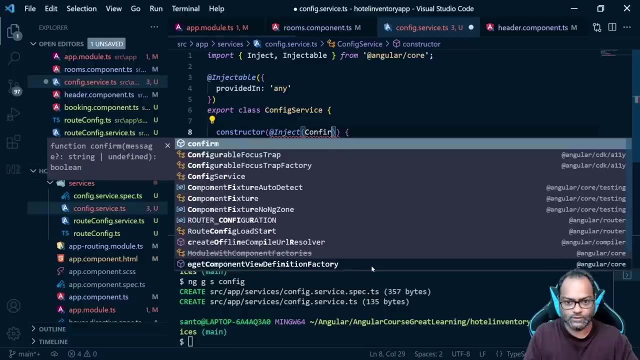 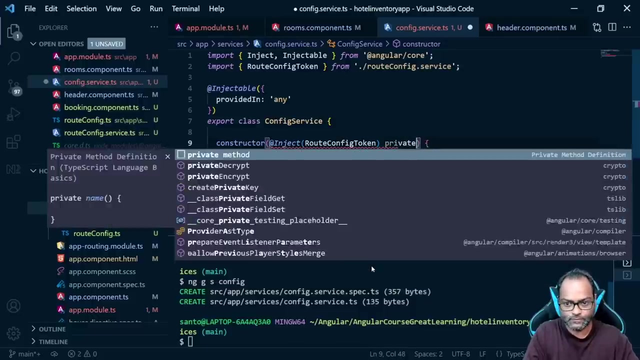 And we will be using this route-config-token. Let's go ahead and use it inside the config service. So now we know how to do that. So we'll say: inject And config Route-config-token, Run in back config-token. 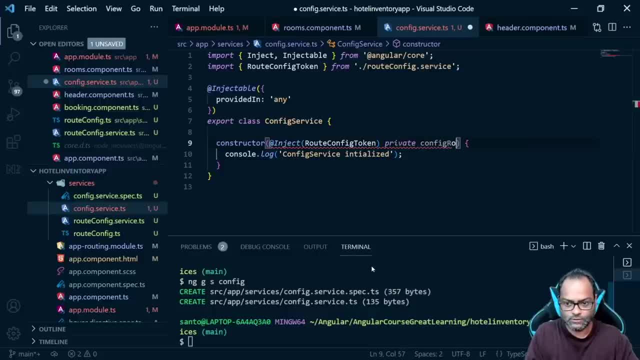 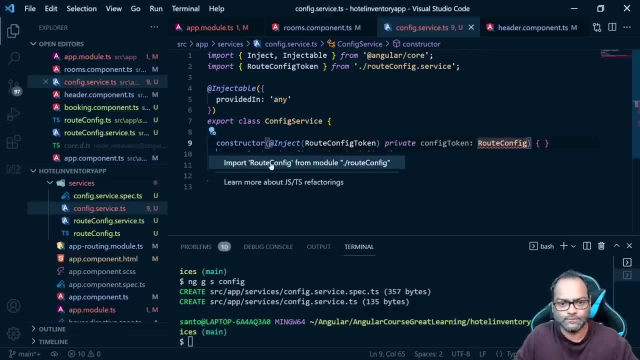 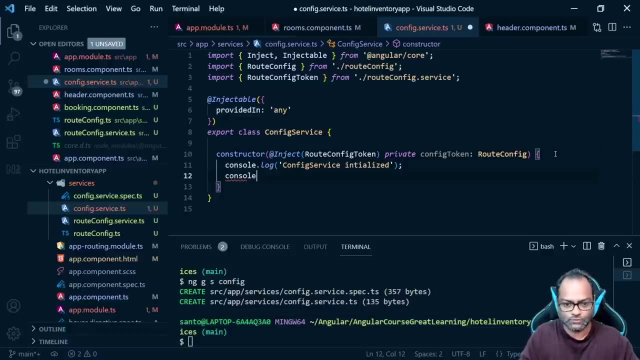 And route-config right, So we'll just import this as well And let's print the value. I think this is remstrom consolelog. This is route-config-token. Let's run Rectrum consolelog- Resort-config-token. Let's verify this functionality as of now. 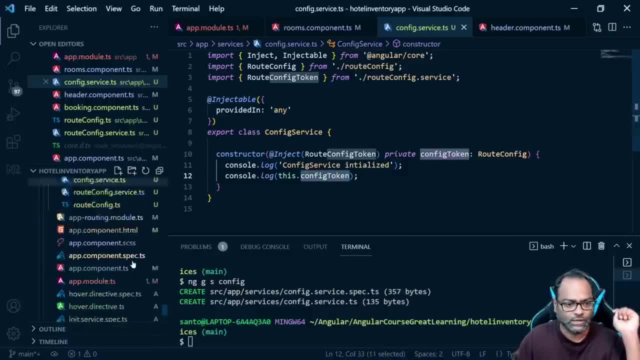 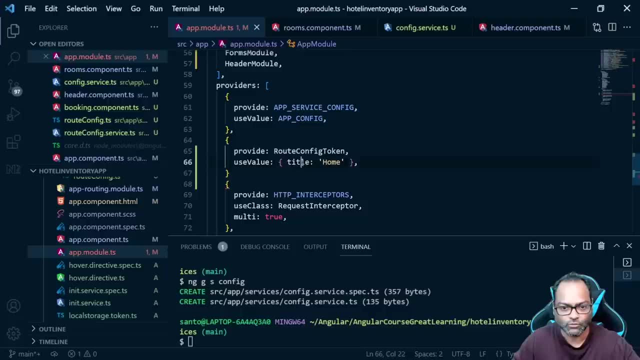 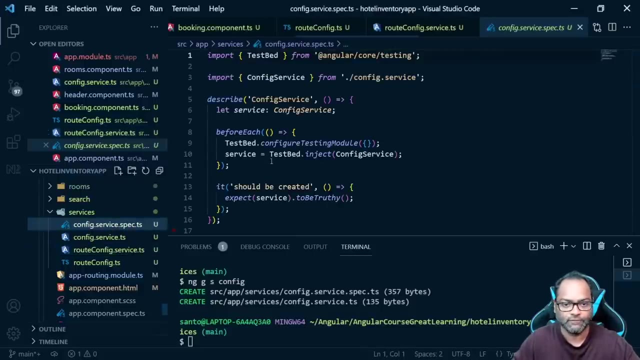 So we have this service, which is now injected in. So what we did is we created a config service and we created a token. We provided a value to this particular token, We said title is home, And then we use this particular thing in service and we are just actually logging the top token. 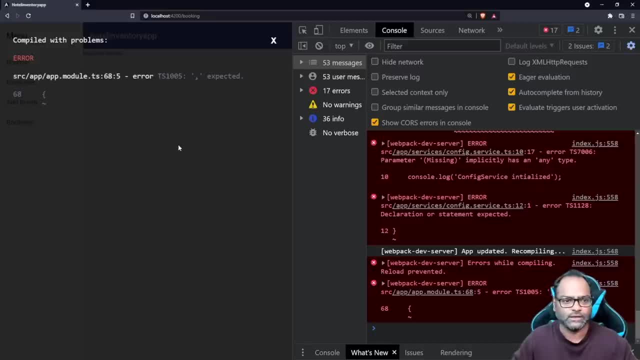 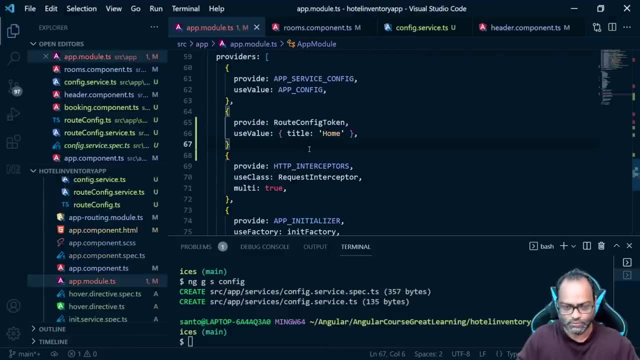 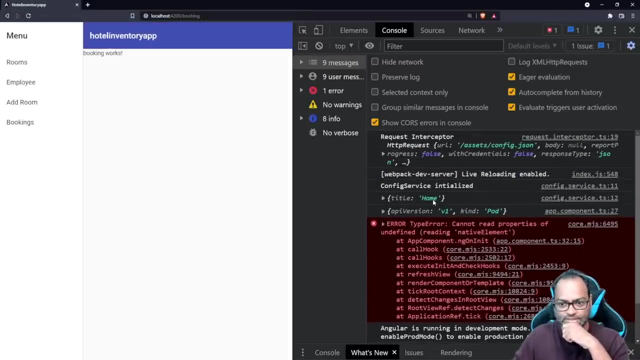 value. Let's see what we have done so far. And there is something unexpected, which is appmodelts, line number 68.. Let's see, probably I just missed a comment, Let's go ahead and see. So what we have here. so config service right now has a few instances, right. 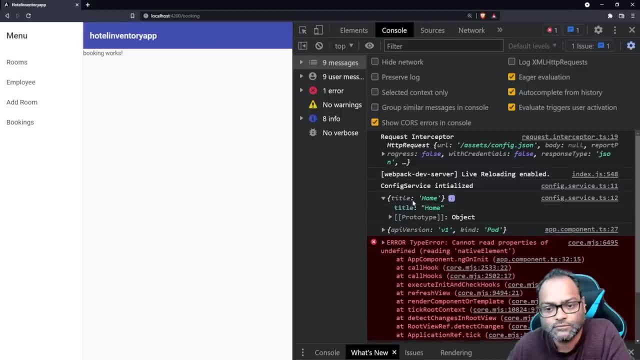 So we have this config service initialized and then we have title home. You must be wondering what we have done- I mean, this is something which we have already done- again why I am covering this thing again. I mean, we know how to use. 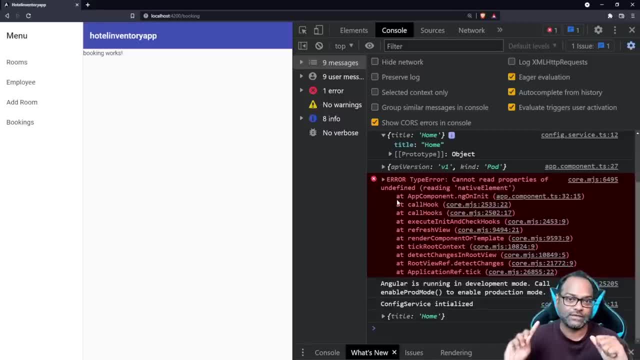 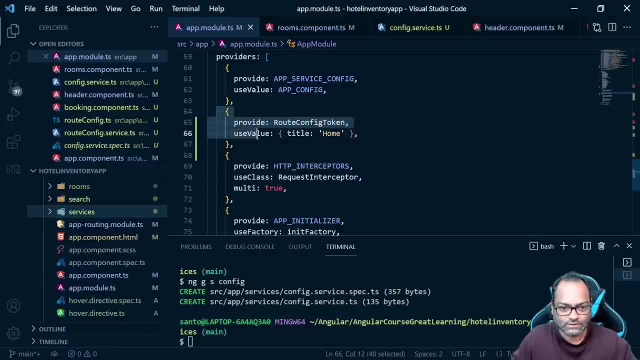 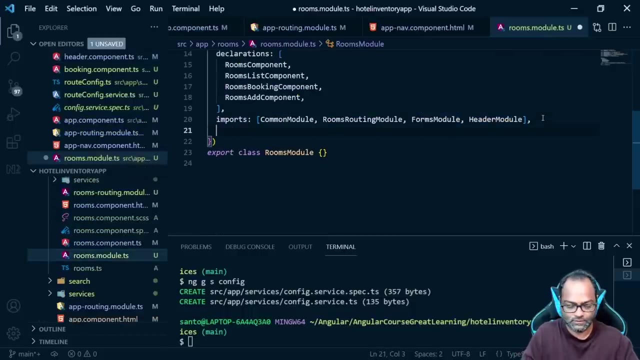 injection tokens, but there is a difference when you use provided in any Here. let's try to pass this value to rooms module And what we'll do is provide this and I'll say: title is room. So remember, right now we are saying there's another, we are just changing the title. 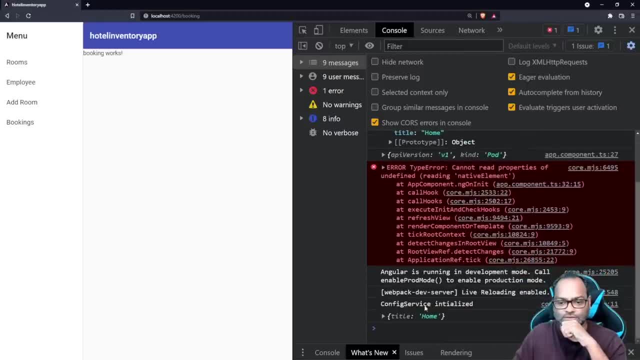 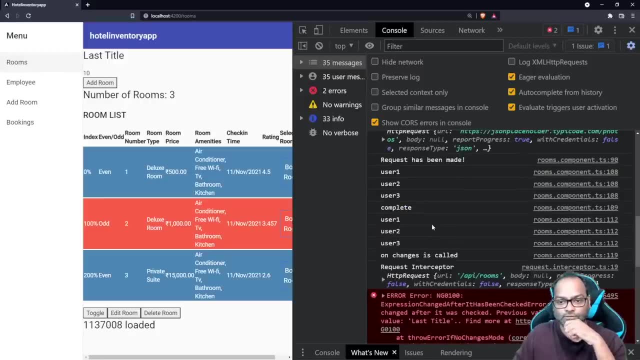 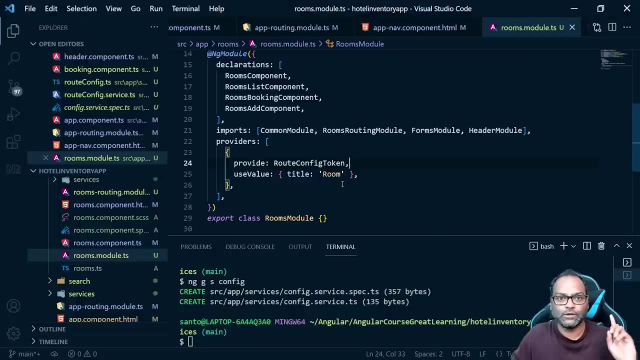 Let's go ahead and see. So we have title available as home, available here, right. Let's go to room and let's see what is the title available right now. So we have title as room. it changed. Let's switch back to any and let me show you what will be the value in case we use any. 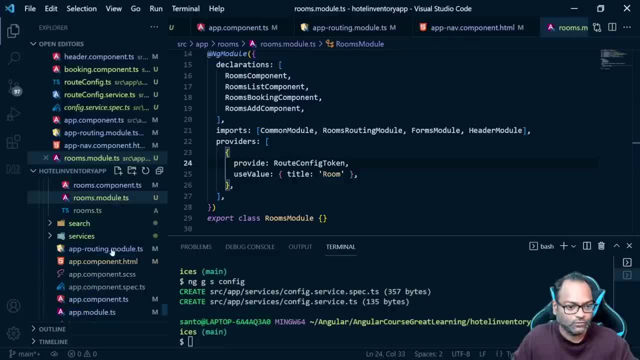 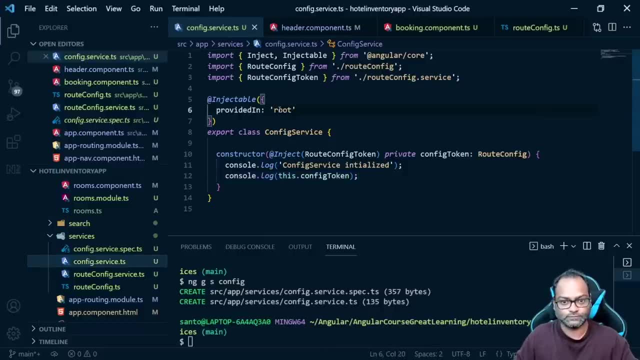 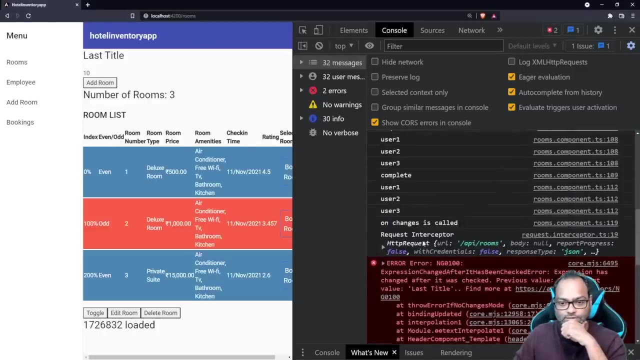 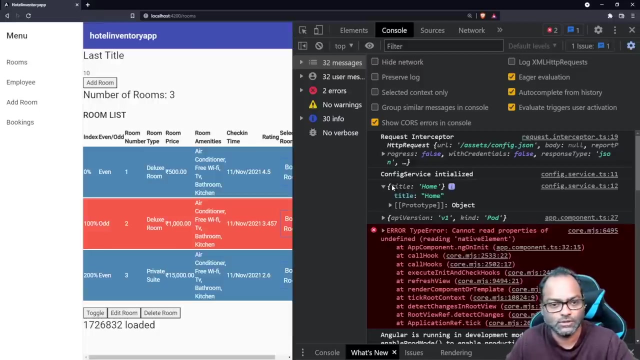 sorry, We use root. So let's go back to the rooms, sorry, config service and change this to root. And here it is, So you will still get for rooms. even for rooms, we are getting the value as home. Let me show you. 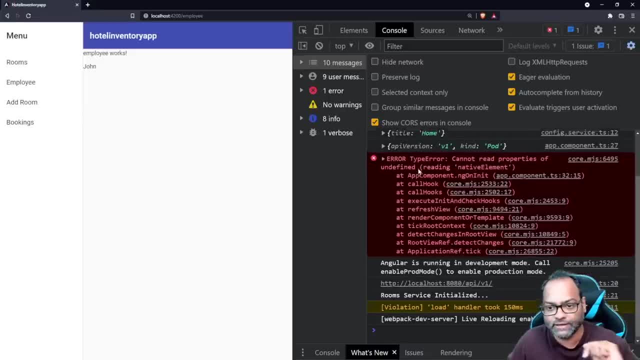 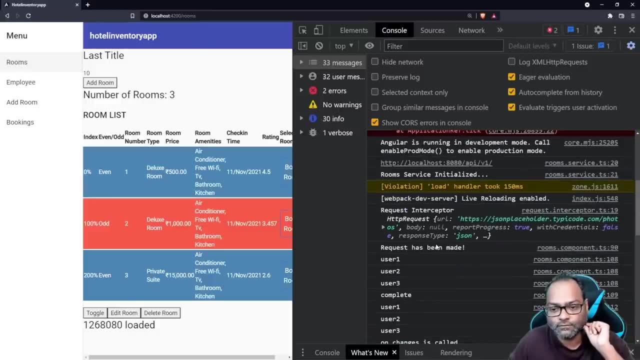 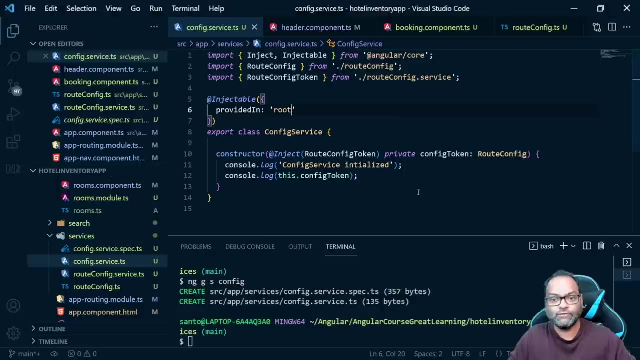 I mean probably let's move into another module so we can see the value. So we have this home, of course, which makes sense. Click on rooms, We will still end up with home. why so? Because when we say root, it's a singleton instance which will be available when we 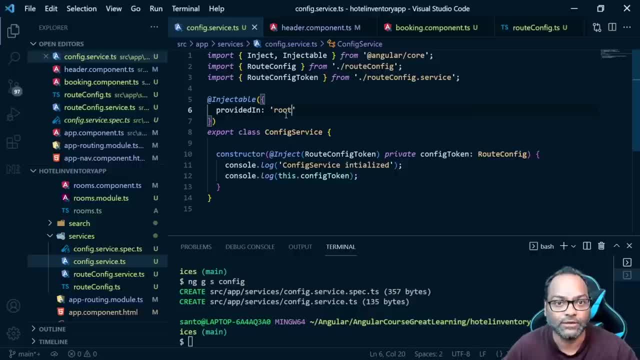 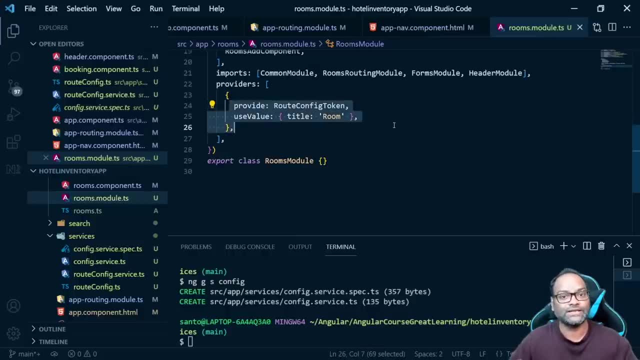 are saying any, it will create a new instance for that particular service. So we ended up with the new value which we registered into the module. Otherwise, we will just get the previous value as which was Okay. Add it into app module. 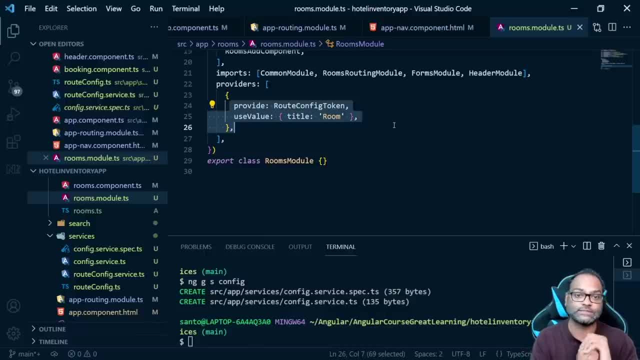 Remember this. this is really interesting, Interesting thing which landed in angular nine and it's really useful. So a lot of developers don't know this functionality, which is able, able but can be, can be really useful in case you want to actually go ahead and pass some other configuration. 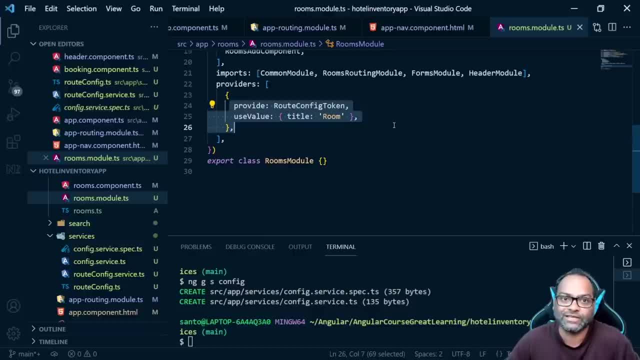 Which is which? are you want to overwrite some configuration inside any of your lazy loaded module? Very interesting use case. So, as I said, my friend has also been covered, So we will just get this, Okay. Yeah, this is pretty easy. 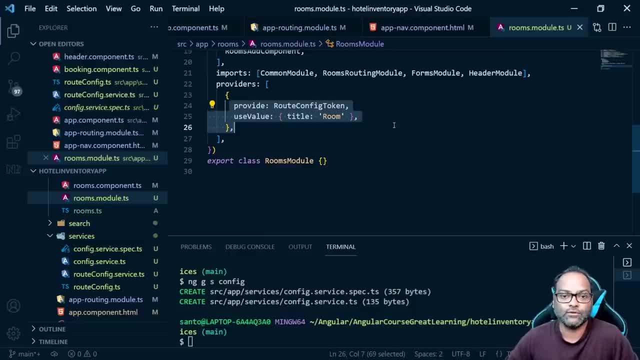 So that was a little bit of a story. Sorry, sorry, I'm sorry, But you guys are doing it. This is a little bit of a story. So it's a little bit of a story. it in very much tailed way in his book and you can also go through that use case as well. so this is. 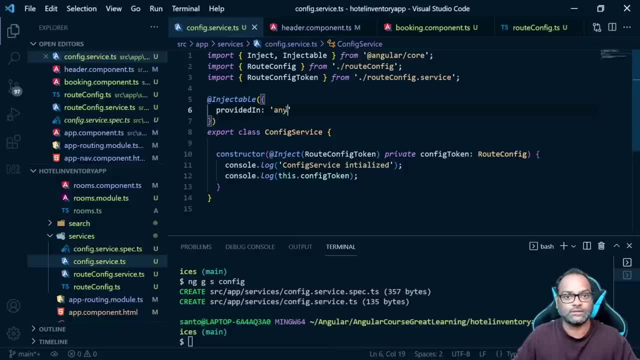 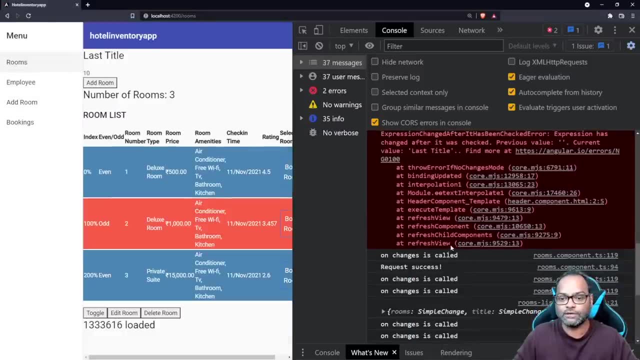 it about any now i'll just change back to any, because this that was the purpose of having this particular service and we are done so now we will end up with whenever we click on rooms. we will end up with configuration as title room. you can pass any configuration for separate or you can. 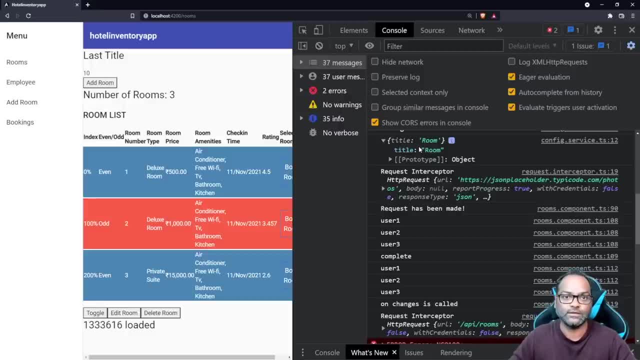 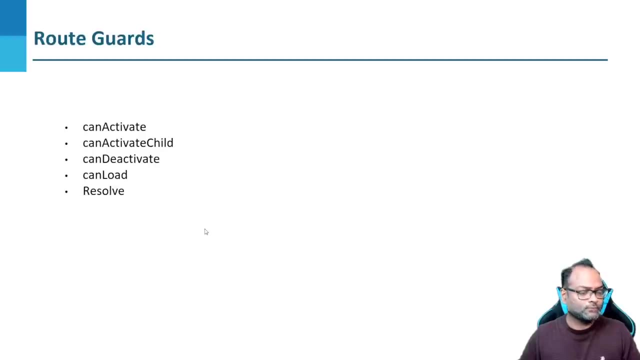 just overwrite the configuration for your lazy loaded module using in. so we saw both the example using just a service, how it behaves, and then inject. we added injection token to show you how it behaves in case we pass an injection token. let's go ahead and talk about route cards. so 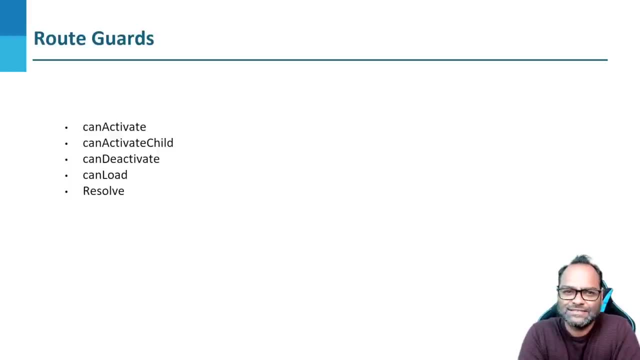 as per name suggests. right, it's cards. what? what you understand by cards? so you have many type of cards and you might have seen you in your real time or real life as well, right? so let's say atms, they have guards, banks, they have guards. what they are trying to do, they are trying to secure. 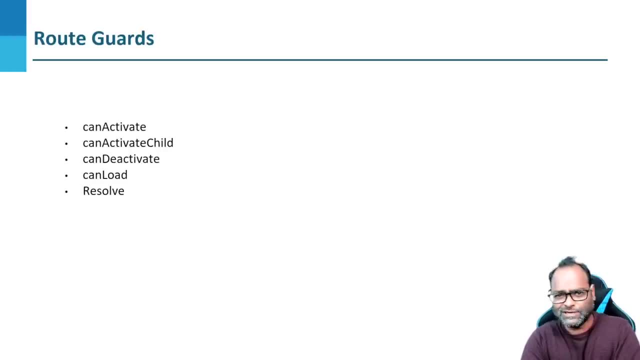 something, of course, in that case it's money. so what route guards do? so it means they, these guards, are actually trying to secure route. but how so? there are multiple guards which are available and they do different stuff, so we will go through one by one and we will talk about resolve guard at the 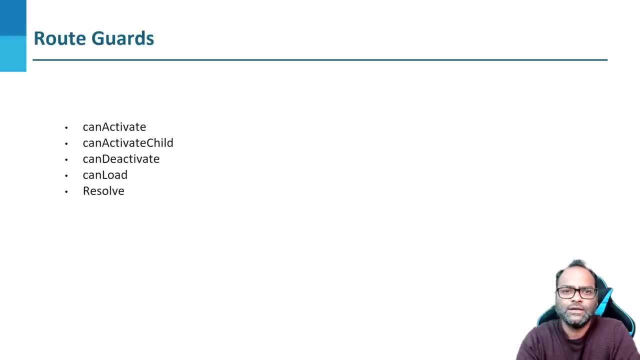 end. before and before we talk about resolve guard, we will create our booking form. finally, and we will fix the date picker issue which we have in our earlier form. right, we, if you remember, we created our rooms and rooms form and we said, okay, this date time doesn't work, then we will be using the angular material date picker. so we will fix. 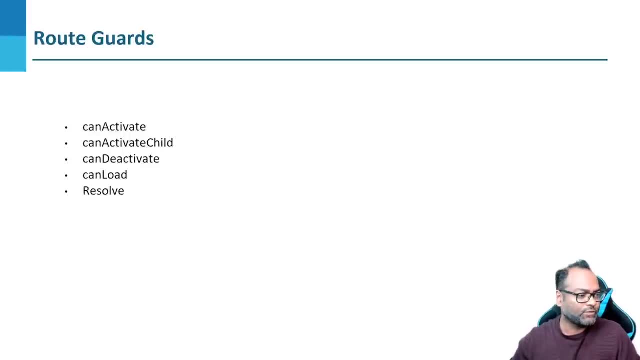 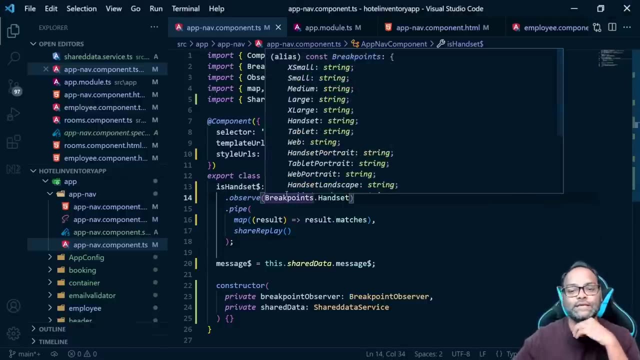 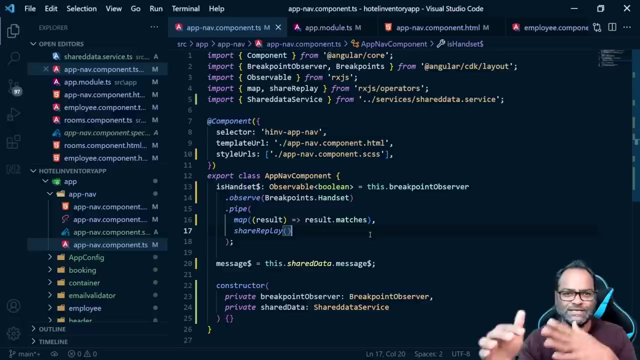 that as well. so let's see how route guard behaves. but before we go ahead and talk about how route guard works, we need to understand one thing. we need to understand the routing event. how does your route works right? so we have not seen this. we have seen, okay, how to configure your route, how to 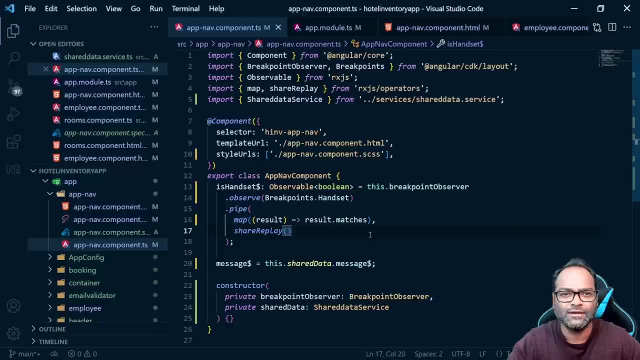 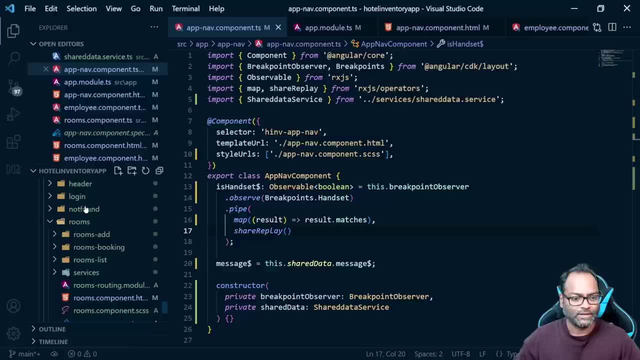 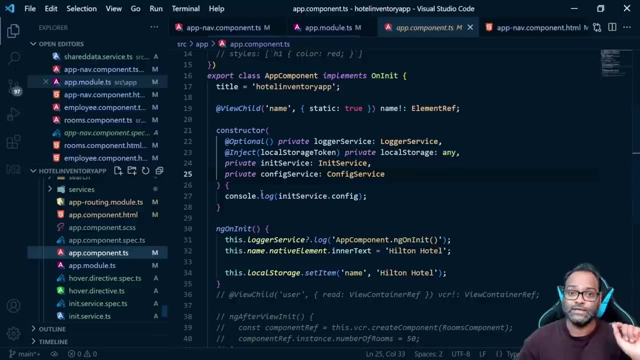 do your default route, how to do your wildcard route, but in which sequence they are called. i mean what happens when you click on route. so let's go ahead and talk about that and to do uh that. uh, we will be subscribing or we will be using the router service, which we have already used, but 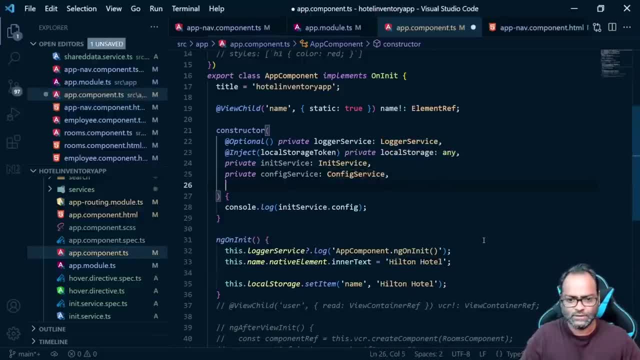 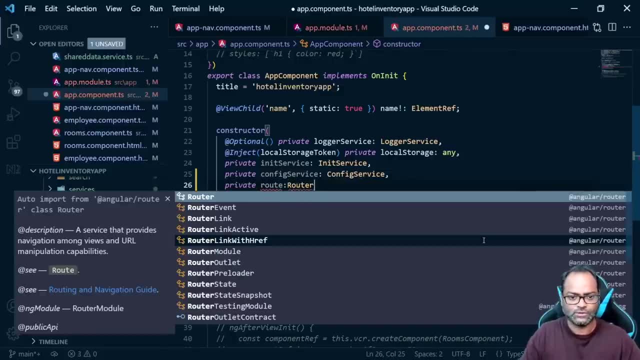 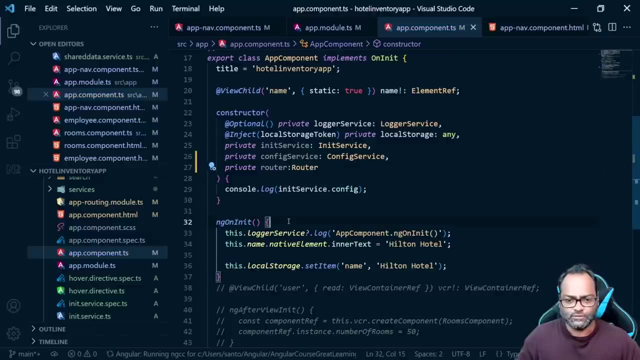 we'll be using some different properties. let's go ahead and see that. so here i'll say private, i'll say: this is route and this is router. now let's call it as a router, right, that makes sense. and now on ng, on init lifecycle, look, i'll say this: dot, router, dot events. 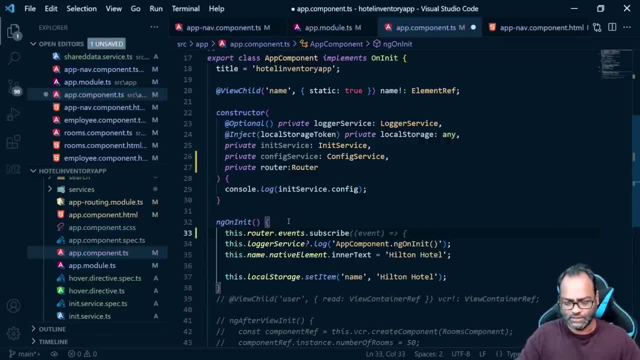 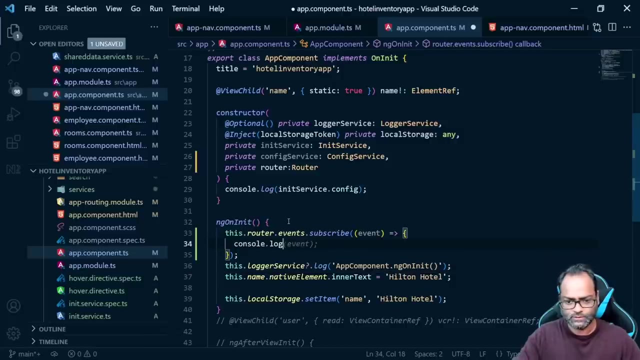 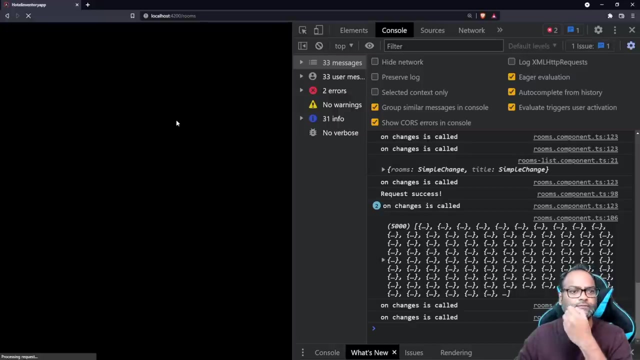 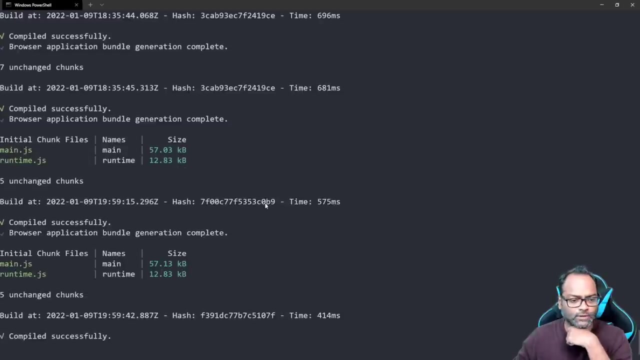 dot and it's an uh observable, so i'll be subscribing to it and then we'll say: this is event, um, um, um, um, and here we'll just do consolelog event and let's go to our ui. let's see if it's compiled. yes, it is compiled and i think there is some debugger which is available. 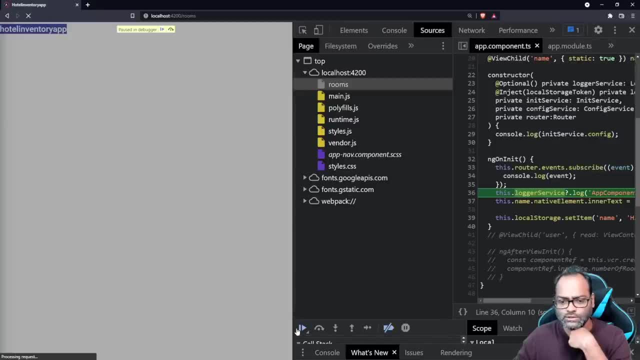 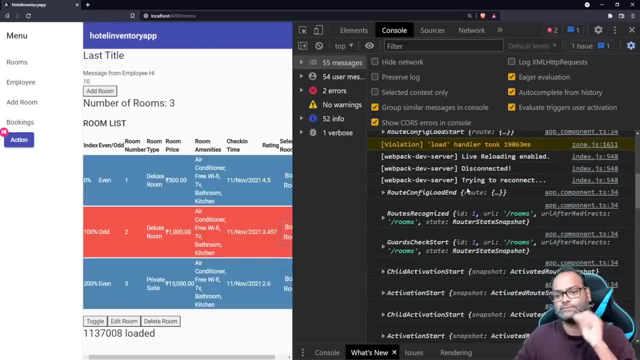 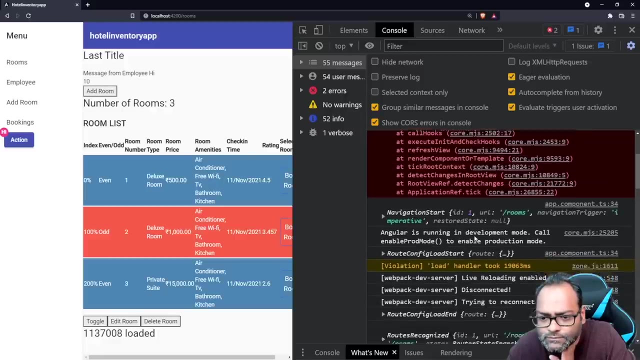 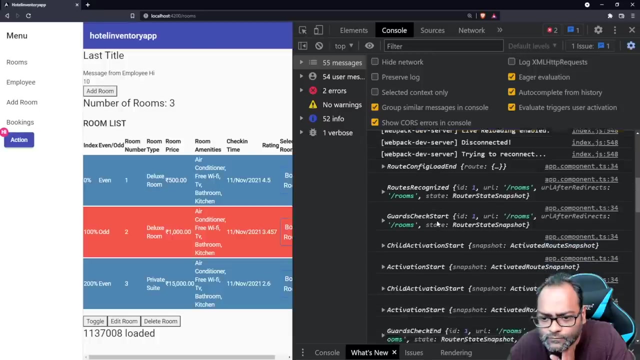 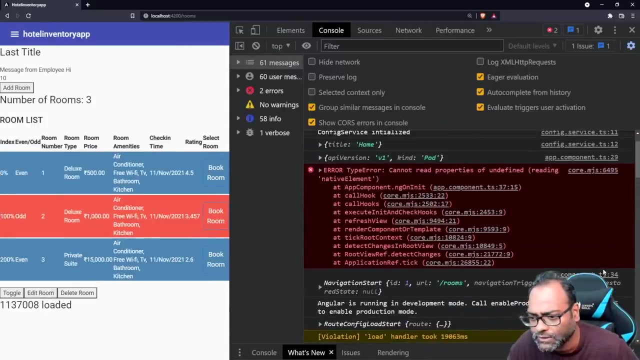 so let's move on. we can just let me just disable the difficult and let's go to console, and here we want to. hmm, so here you can see, uh, line number 34. so let's go ahead and see how it starts right? so when in this, 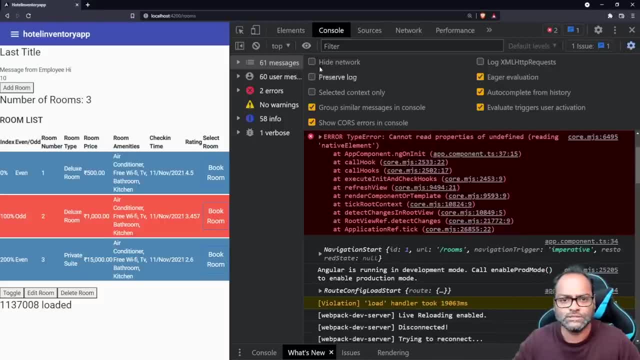 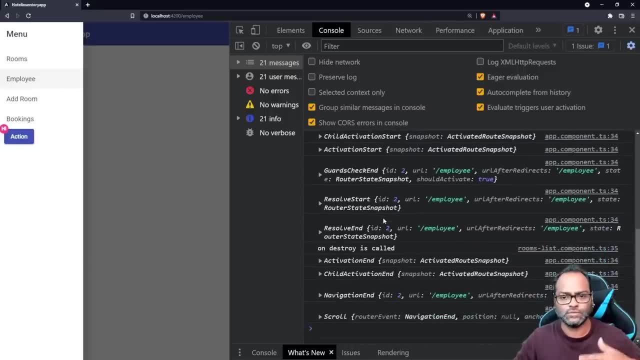 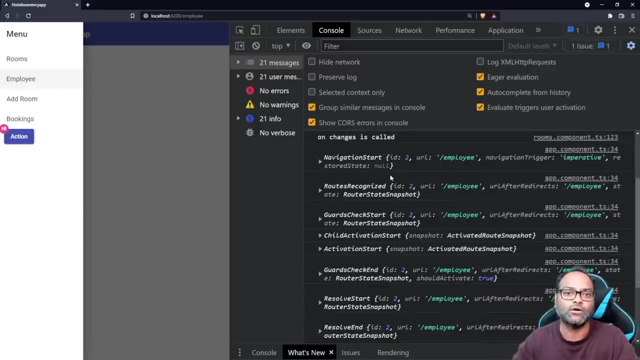 case the navigation happened, if you remember. let me just do this one thing: i'll just remove this and let's go back to employee right. so we have the only route guards or route events are blocked. so there are multiple events which gets fired when you click or in case a navigation happens. 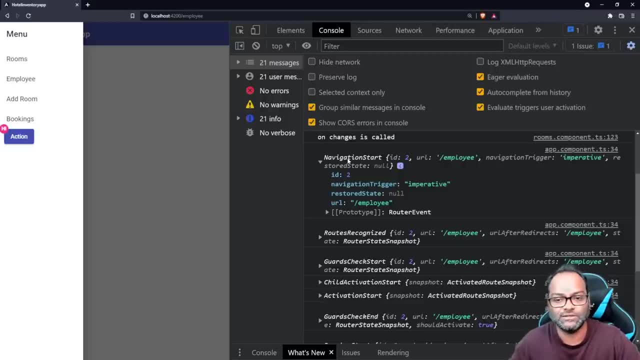 so here you can see. it starts from navigation start and, if you see, there are few parameter which your navigation start has, so it has a url. it has a unique id generated for each and every navigation event which happens. these ids are really helpful in case you are getting some issue during. 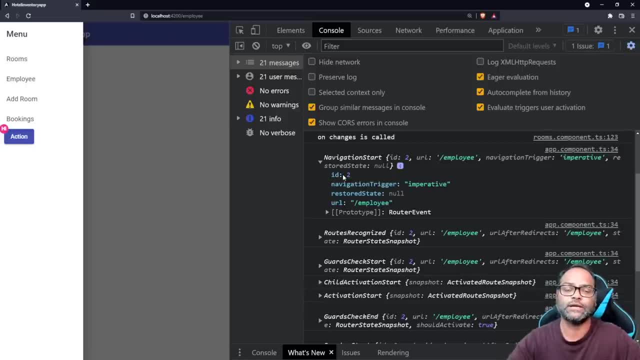 navigation. a common use case or a common issue which we generally get during navigation is, by the time the first navigation gets completed, you are trying to navigate again. so you can only figure that out based on the id so navigation started. then it tries to recognize the route, so it says: okay, now this route is recognized, so i have to uh. 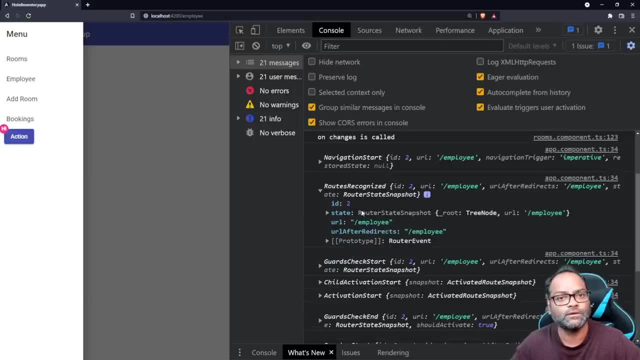 there are some states which is uh available, so remember uh snapshot. that's part of this. you can see router snaps, uh router state snapshot. so you have url url after redirects. then we get uh, get guard check, start, and this is where the route cards come into picture. so 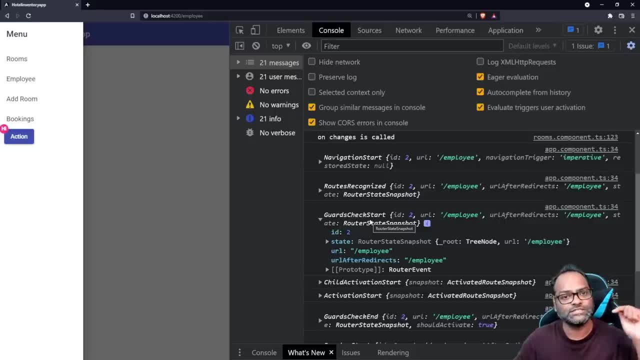 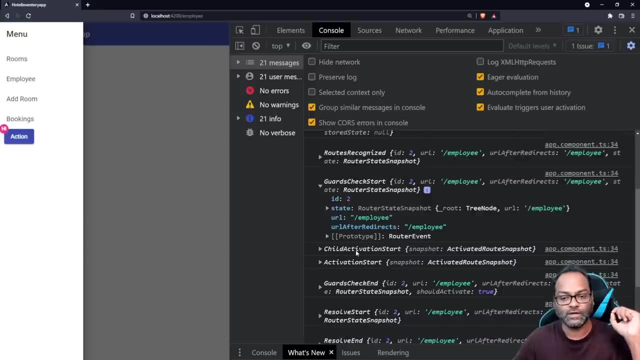 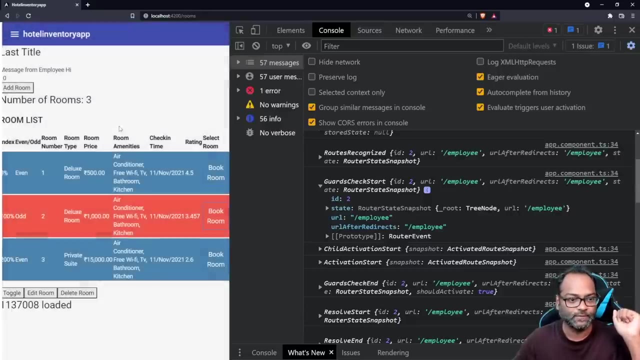 it says: okay, now i'll be in, go ahead, i'll go ahead and check whatever guards you have implemented. so this is where it will start. then it will say: okay, now let me go ahead and activate the child where we have seen the child. so if you go to rooms, click on add room. so this is child, right. so it will go ahead and check if 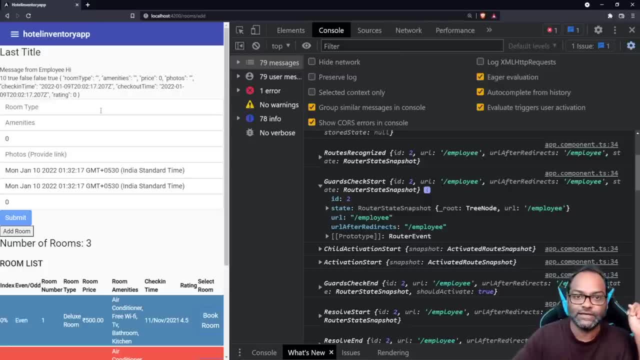 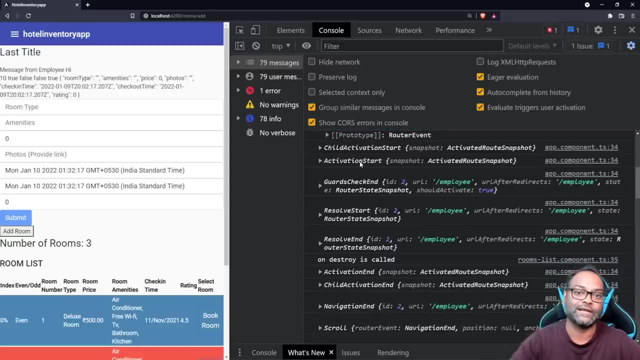 this child. uh, it will go ahead and start activating this child routes. then activation starts. it will say: okay, now everything is figured out, now i can go ahead and activate this particular routing or route. now here, all the guards have checked, all guards check have ended. so it says: 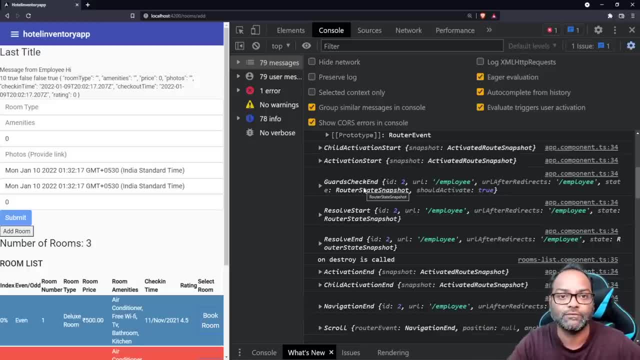 okay, now it's fine, everything is okay, all guards upset. so all all the guards which we have implemented. they are saying it is okay to allow this particular user to enter into this particular route. god's check-in right. so nowadays, when you try to enter into bank or atm, what they do, 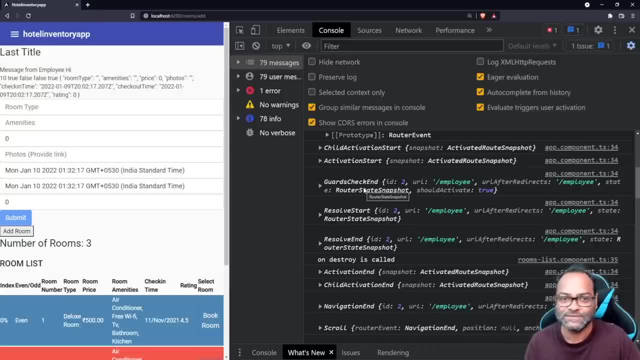 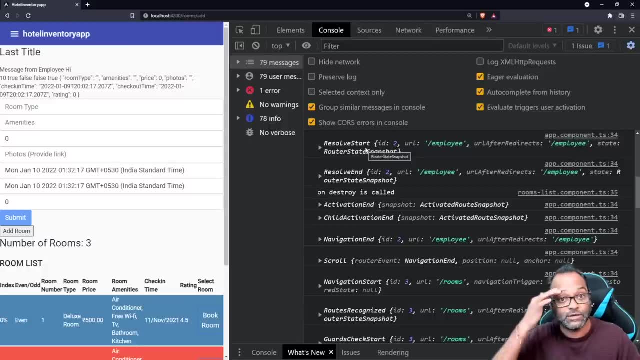 they check your temperature, they try to see if you have any symptoms, right so, and then they allow you. so that's where guards check end. then it says, okay, now let me just resolve, uh, this particular route. right, so it will. it will try to resolve this particular route where 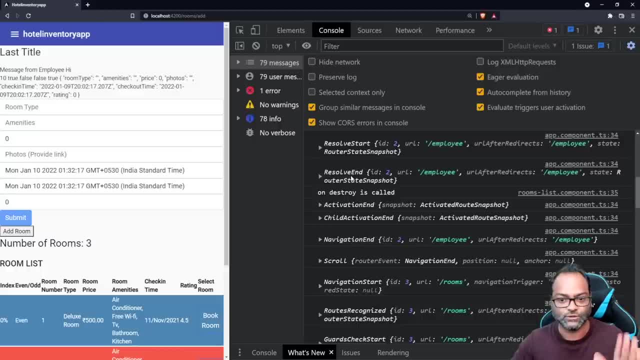 we are redirecting to home slash add. and then it says, okay, now this is also fine, resolve ended. then it will call activation ended and then it will say, okay, now, child activation also ended. and navigation. finally, it says, okay, now everything is fine, let me just end the navigation. and, uh, the 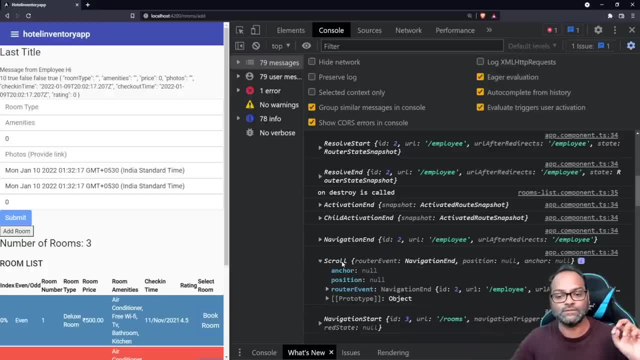 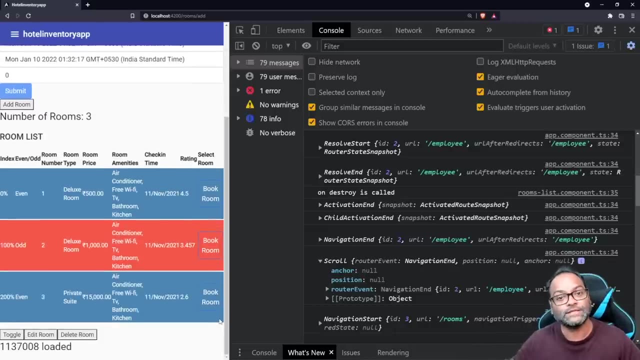 last event which we have is scroll event. scroll event is something which you can use in case, let's say, you click on a url and now you want to scroll your- uh, scroll your this horizontal bar right somewhere, or top bottom, wherever you want to. you can just go ahead and subscribe to the scroll. 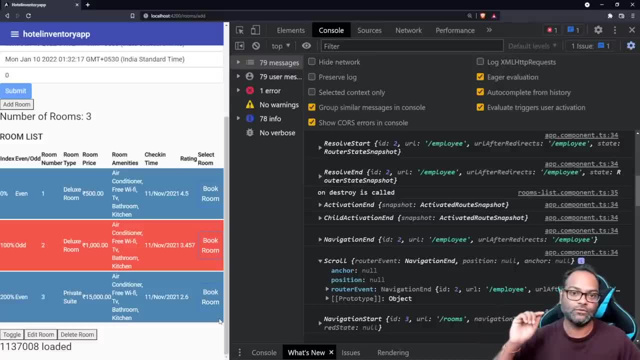 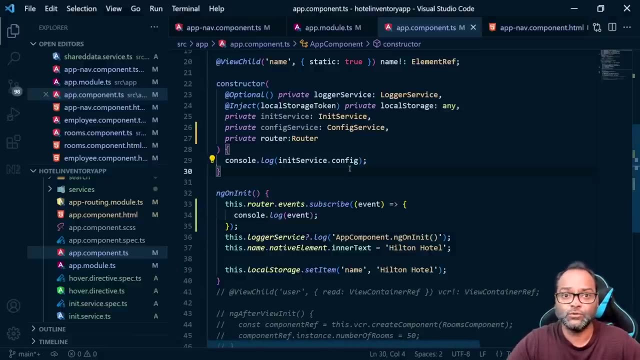 event as well. so this is related to this is related to your router events, how they are called in sequence, and now we will go ahead and talk about the route cut. when working with router events, it is also possible to listen to a specific event. as we saw, there were multiple events which were getting fired right, but in case i want to, let's say: 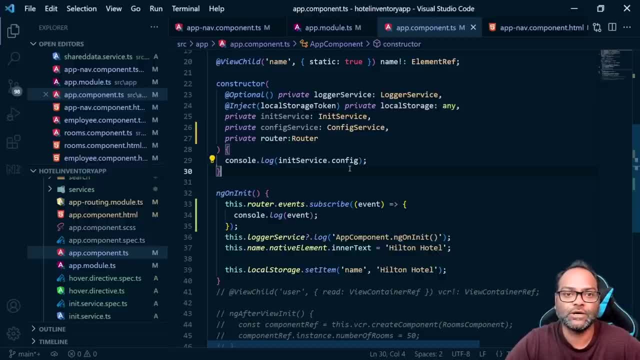 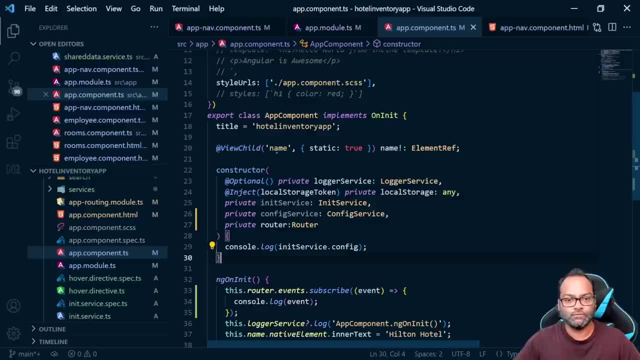 show a loader when navigation start and show up and look- i mean, remove the loader when navigation ends- how you will be able to do that. so we can actually achieve that by using something like this. so i'll just rewrite this code, or let me just keep it here so you can. 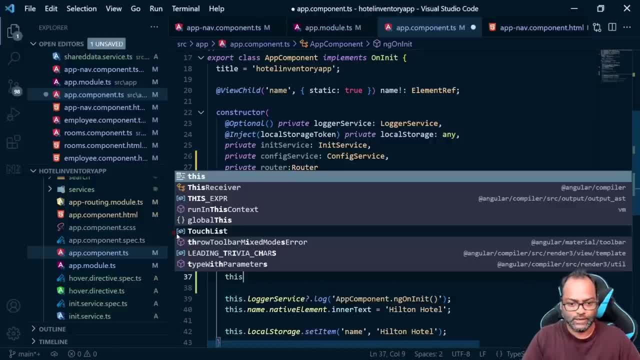 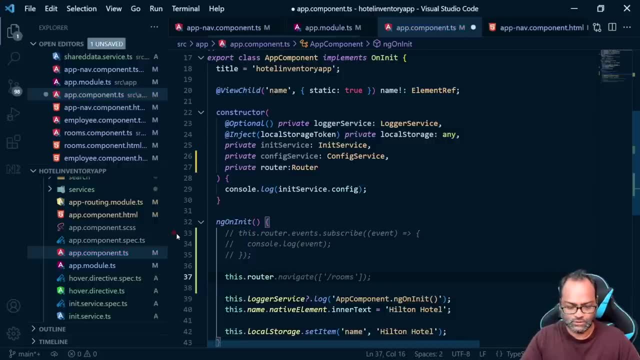 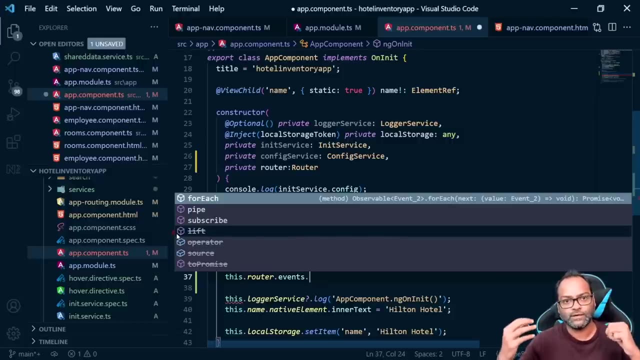 start this while revisiting the code and let's try to listen to the specific event navigation. start navigation and that's it. so we'll say this: dot router, dot. events, dot. now, as we said, we need to listen to specific events, so i don't want to go ahead and listen to all the events and then filter. 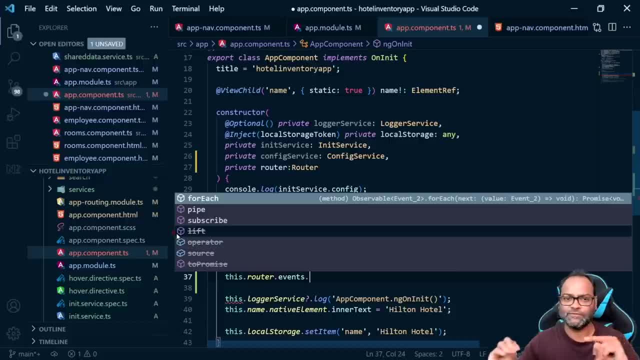 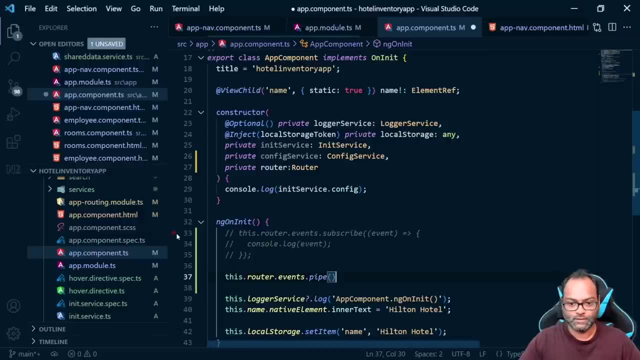 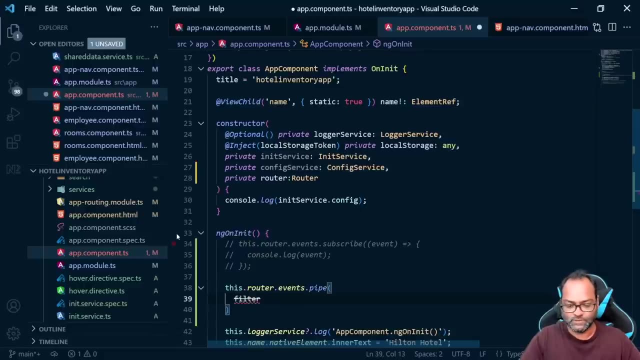 out. we will be using rxjs. remember, little bit difficult, but with some practice you will figure out how to use rjs. so here i'll be using pipe and inside pipe i'll be using filter operator. so you let's see if this- yeah, it is from rxjs and 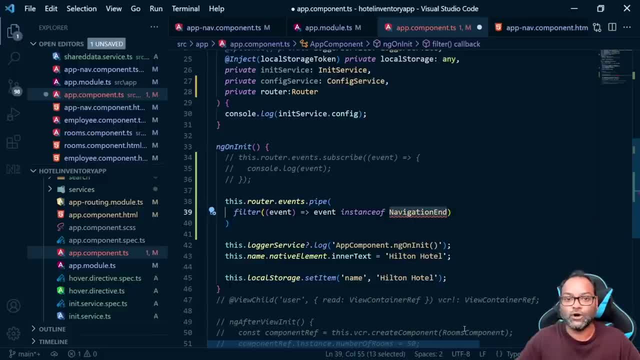 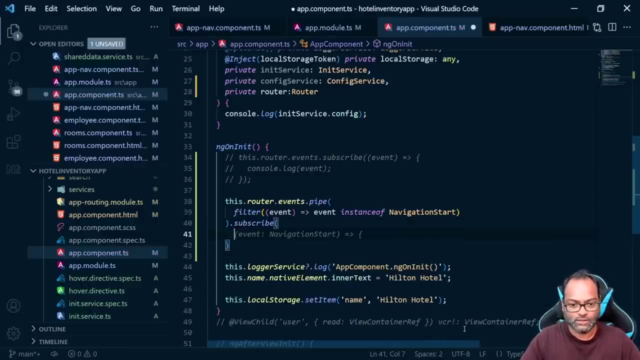 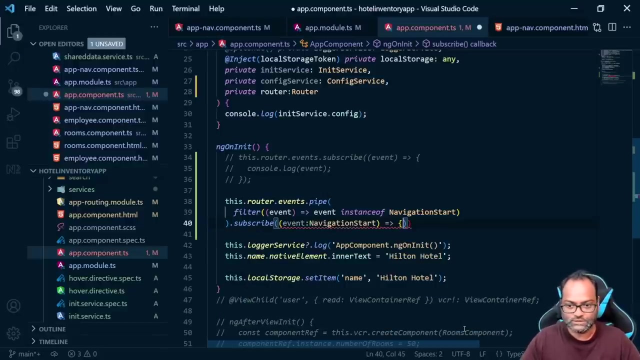 in filter i'll say this event, which is instance of, i'll say, navigation start, right, so i'm just listening to the navigation start event and then i can subscribe. and here let's say console, sorry, i'll say: this is uh, navigation start and we can remove this. i think let's see. 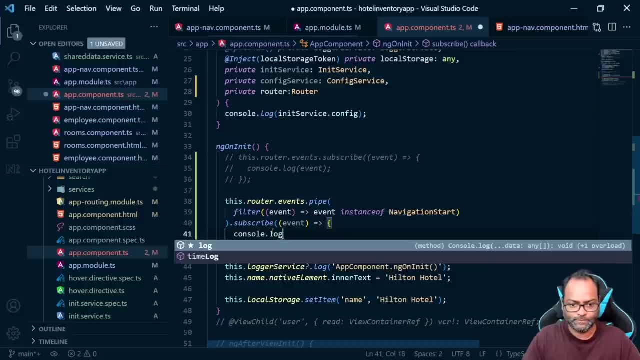 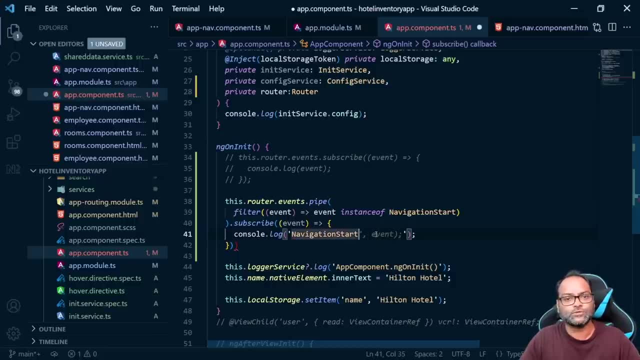 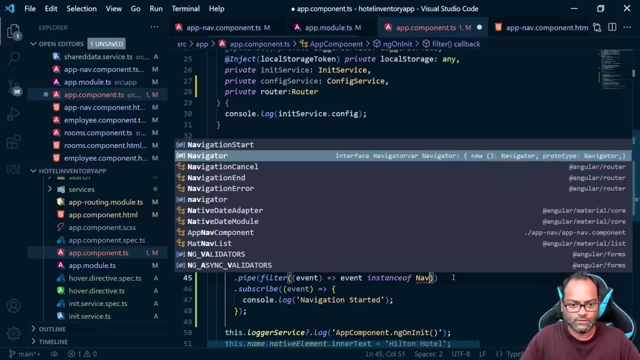 and we can say: console, dot, log. and now you can actually write a code here to show a loader: navigation started right. and then i can just use another option, like already done. so just paste the location name and this given, where i'll say navigation end and i'll say navigation completed. 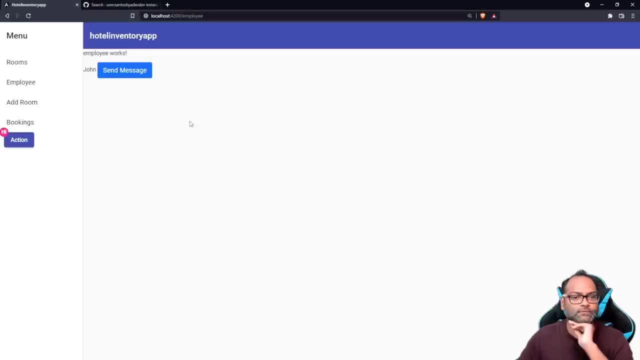 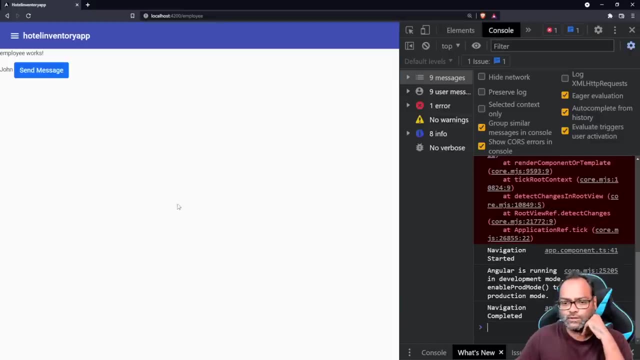 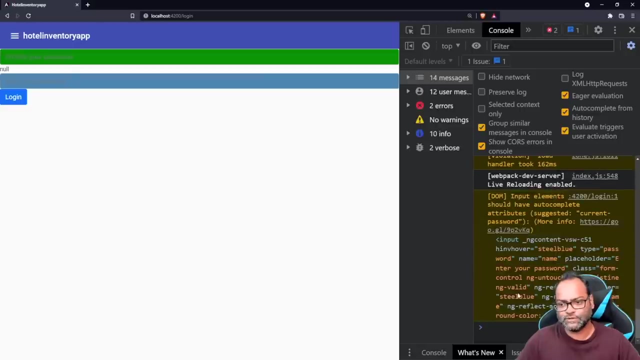 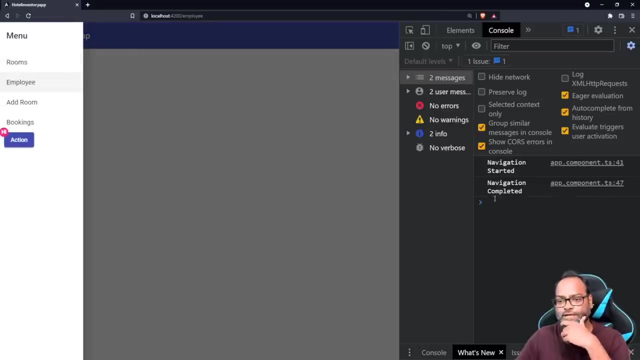 let's go ahead and see if it works, right. so let's inspect, go to console and let's go to to default route first, right? so we can just remove all the comments which we have and let's click on employee and you can see navigation started. navigation completed. 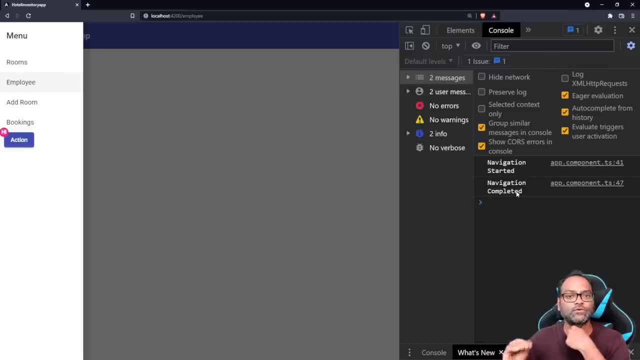 so we are listening to only these two events. so this is how you can filter out the other events in case you don't want to listen to them. so just to give you an idea how you can actually achieve this as well. now we understand how the routing 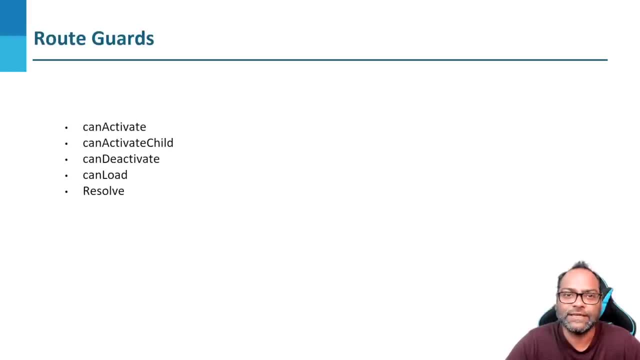 event works and how we can listen to specific events in case you want to. so now let's move on to the route guards. so we we discussed what guards are, what route guards are, and let's see what these different guards do, right? so, as you know, in banks also they are. there are. 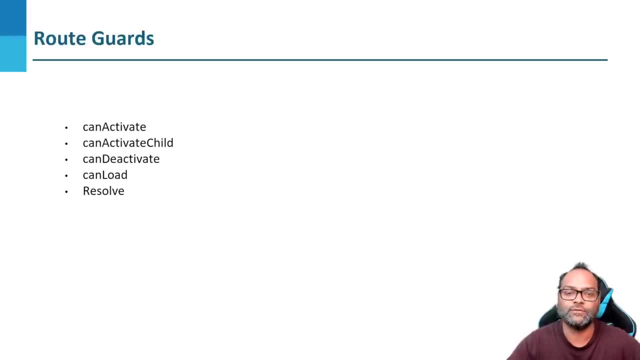 different guards in case, uh, there is a guard who is like standing in front of your bank there, if there are, there are some lockers or some, uh yeah, some lockers in bank- they have different guard available right to secure that that area. so, similarly, router has different guards for different uh areas to secure. so let's start. 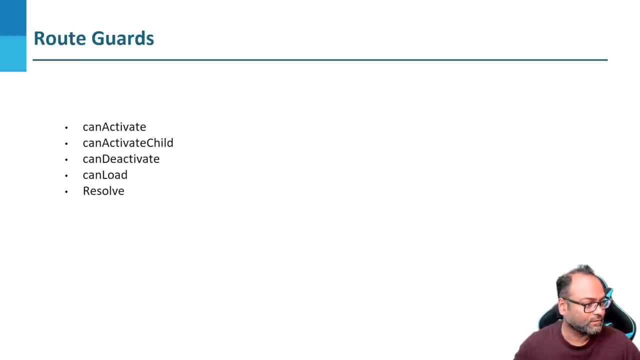 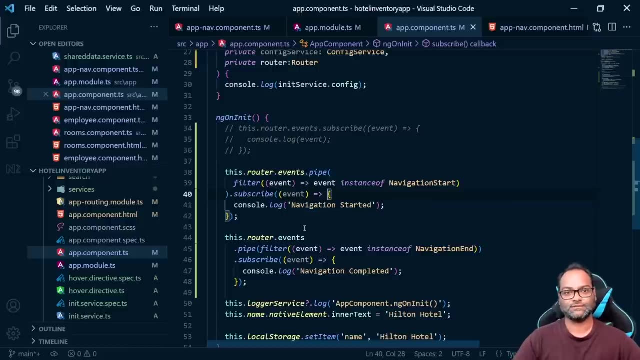 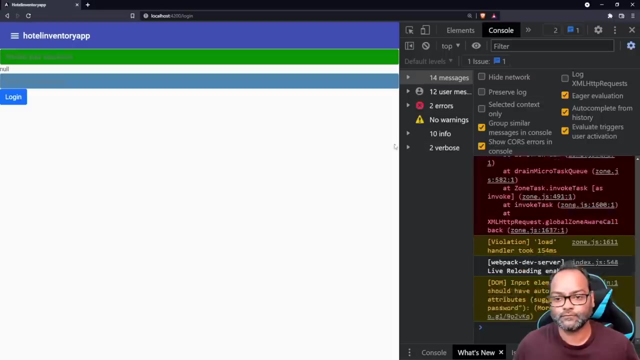 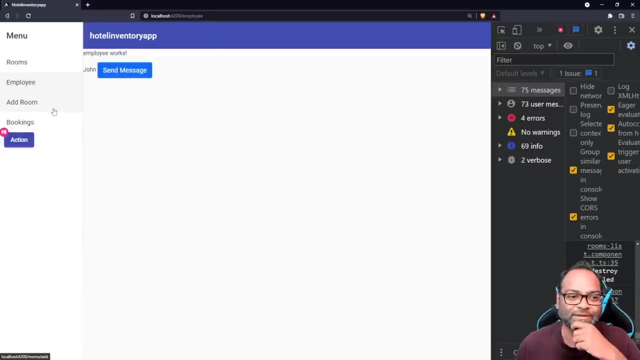 with can activate and for can activate. we actually have a very nice uh use case already. let me show you. so remember we already have this login page. but is this login page use useful? yes, there is no. this is like some uh guard who is standing in front of bank but he is not checking anyone. 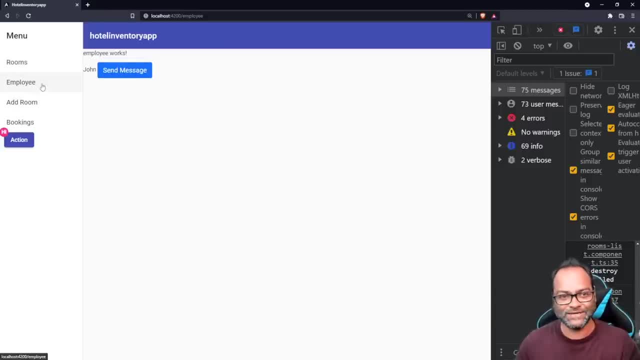 he is just letting the everyone go, so it's pretty useless, right? so here, uh, what we can do is the can activate card. let's relate to can activate card. so, can activate cards. uh, guard, actually tries to see if i'm uh sorry, if i am as a user, of course, at the end, as the as the end user. 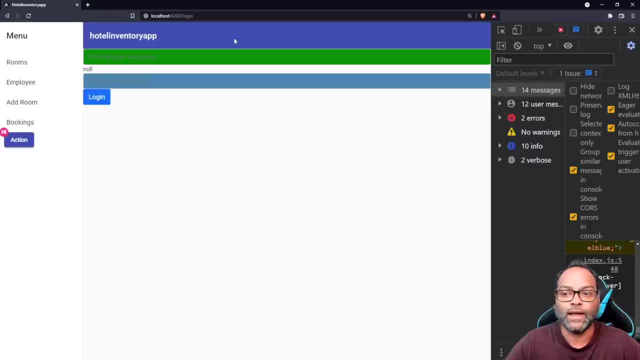 is a valid entity to access this particular route or not. can i activate? can i activate this particular route? that's what can activate is all about. it means that guard is actually checking if no one has fewer right. i mean, that's what they are supposed to do in in days of corona, so they're 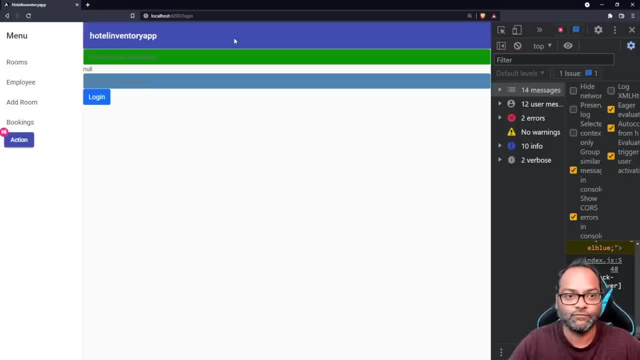 supposed to check your temperature and everything. so if you have a few fever, they are supposed to let you go and the same thing will- uh is uh. same thing can activate will do for us here. so, in case we are logged in, we should be able to access the different routes which we have in case we are not. 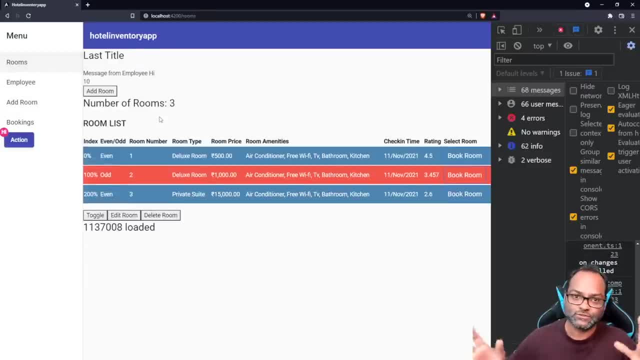 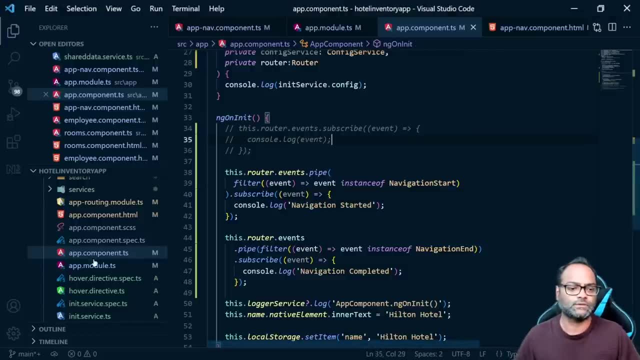 logged in. we are not supposed to do that. so, based on some conditions, you can secure your road. let's go ahead and create cards, or we can do that, so i'll just. what we will do is, as we are supposed to write few other cards as well, i'll create a few other cards as well. i'll create a few other cards. 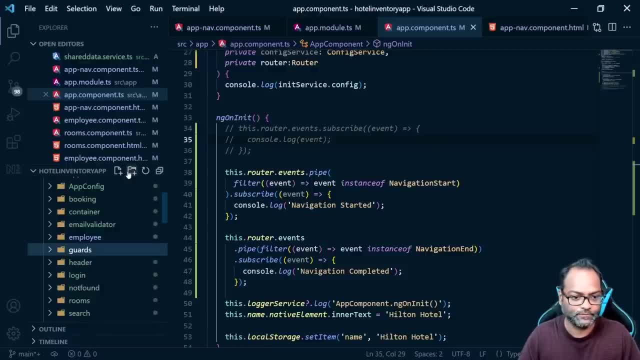 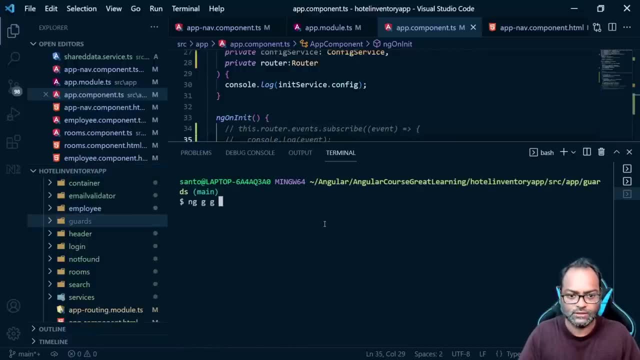 a new folder- i'll just call it as guards- and let's go to terminal and you can see ngg card. so nggg and i'll say this is login guard, as we are supposed to check if the user is logged in or not. i mean, it can be anything, right, it can be, uh, your scenario. so, uh, we have, can activate, we. 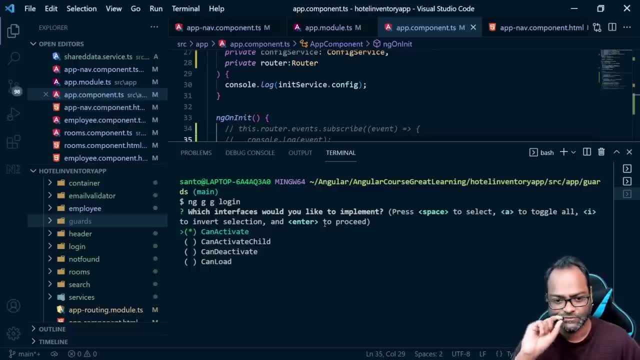 will be using can activate child, but we will be using it for rooms, so we will not add this can activate. we will use it for another form which we are supposed to create and can load. we will use this one so we can select. you can select which of these router guards you want to implement. 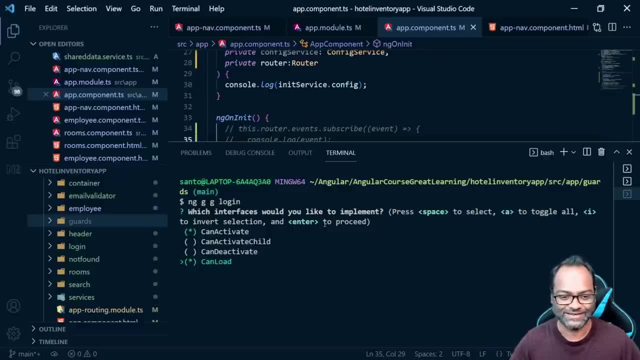 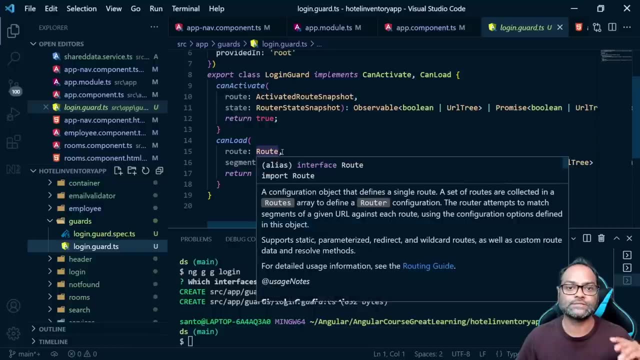 wondering why resolve guard is not there. we'll talk about it, don't think about it right now. so we are supposed to. we chose two guards which we need to implement can load. we will talk about it later but, as is, it is supposed to be part of this particular file. i just added it here. 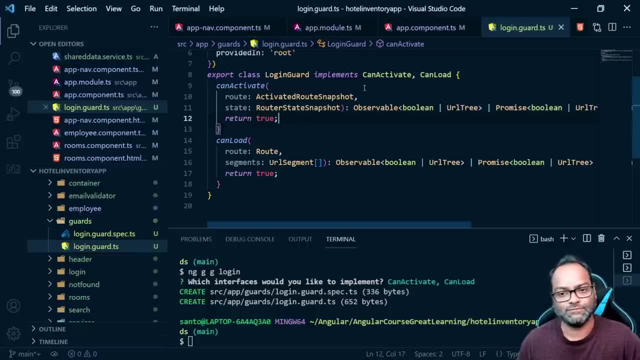 so now let's see. so what we have? it's a interface. it's an interface which has a function called can activate. it gives you some data- we will see what we can do with this particular data- and it returns some parameters. let's talk about this later on. so here, uh, by default. 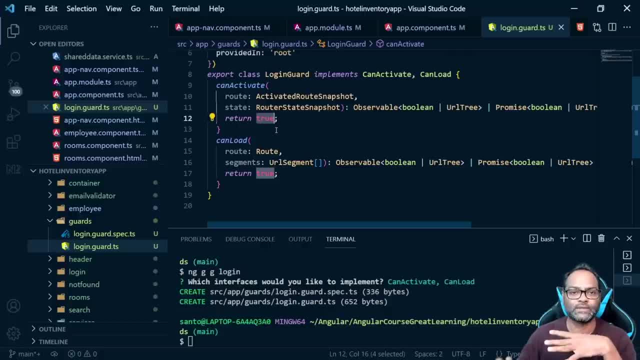 the shroud guard returns. true, it means this is the useless card which we have. so he is just letting everyone go without checking the fuel. so but let's see how to apply this guard right. at least let's understand how to actually put that guard in front of the bank. so here in your routing. 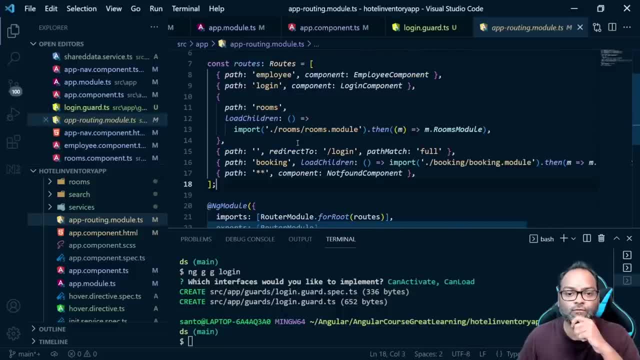 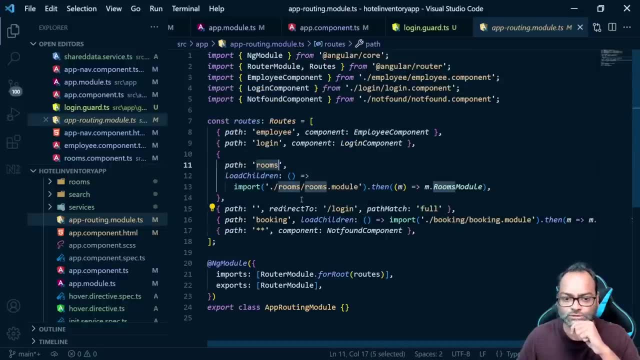 configuration. you can just go to route configuration and you can choose. what are the different areas which we want to secure? so we want to secure employee, we want to secure booking, we want to secure rooms- right, and we don't want to secure login- another if we secure the login. 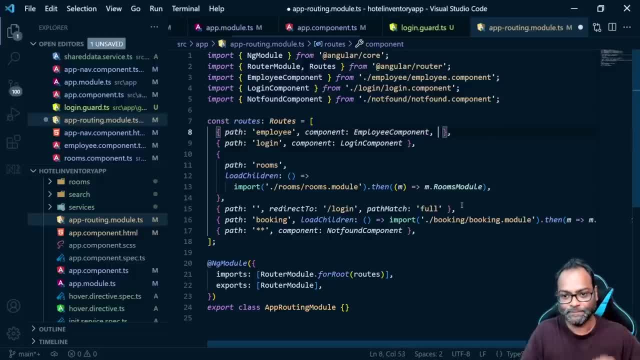 game over, right? i mean, no one will be able to access login. so here you can use, can activate property, and it's an array. it's an array, remember this. it means i can just add n number of guards. so let's say i have a login guard, i have a role guard, for example, there are different types of. 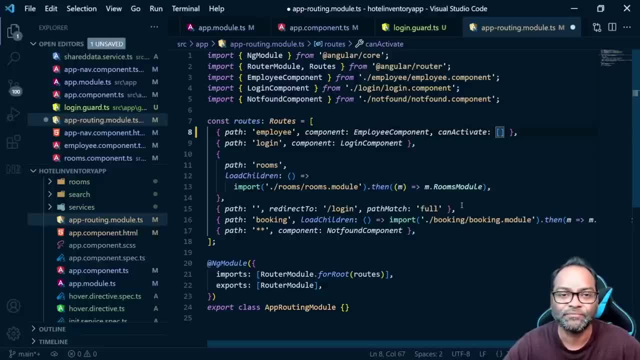 roles which are assigned to access your lockers, right as in. let's say, uh, someone from admin, i i'm not supposed to access the lockers, but someone from the accounting i'm supposed to access the login. let's say, uh, access the locker. so those are. those are the uh criterias which you can put you. 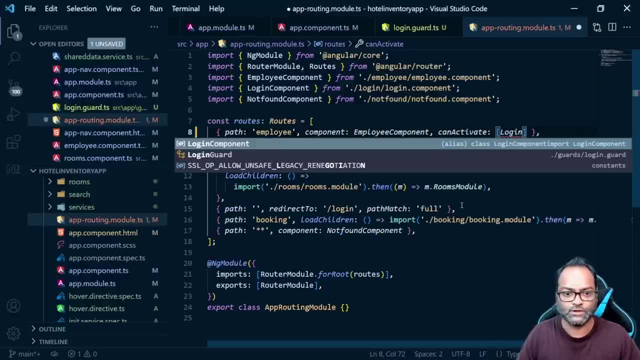 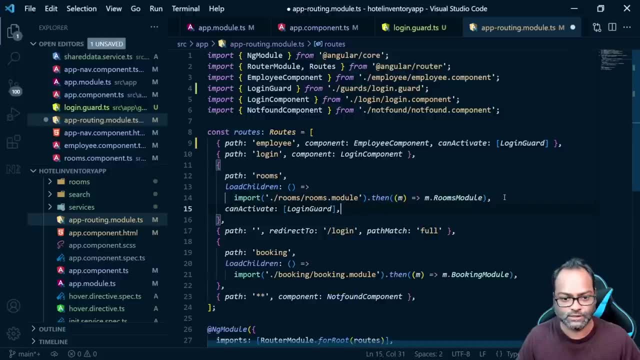 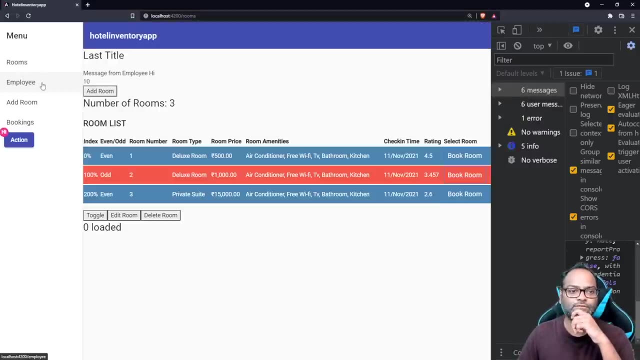 add another card and just add it afterwards. so here we just have one. so i'll say login, that that's it. i'll just apply this to all the places which we have, which we wanted to secure. so i'll say this: you get a guard, you also get a guard, but, as we said, right now everyone will have access to. 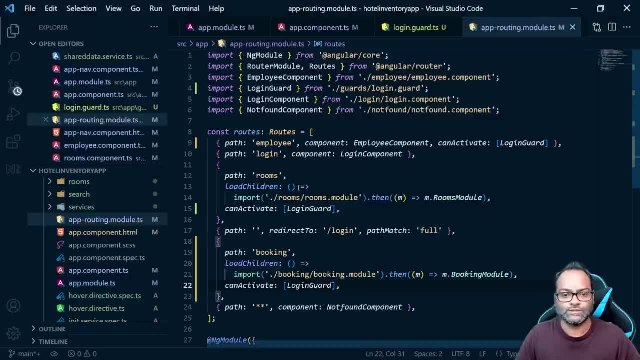 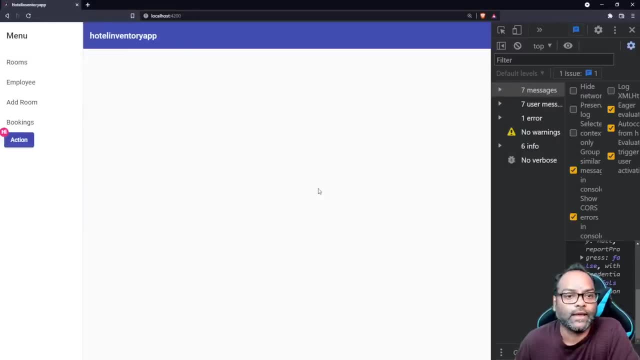 everything right now. let's go back and change that true to false, and here it is: we don't have access to anything- and let's go to login. we should be able to access login because we said, okay, this is something which is not secured as of now. i. 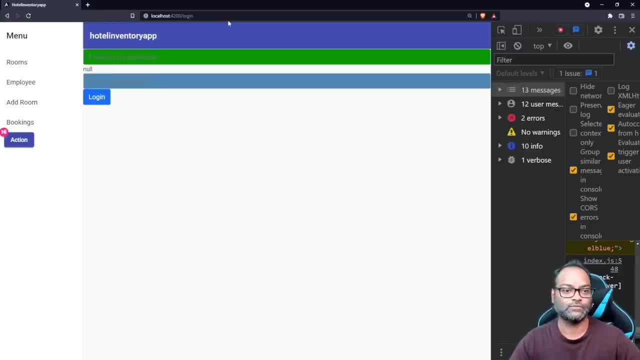 mean there is no guard in front of login, so it works. but what in case? i mean here so it doesn't work for anything else, and even if i try to do this will be redirected to login. but you saw right. i mean, we were on the�� 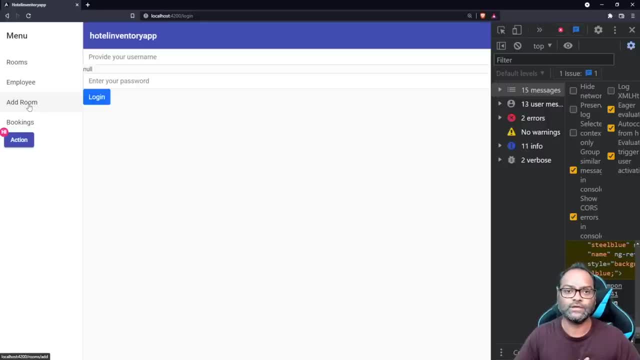 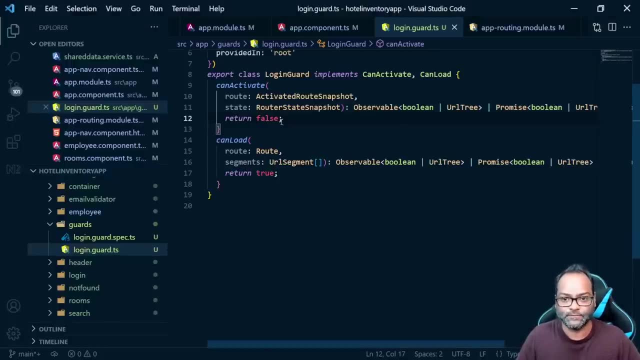 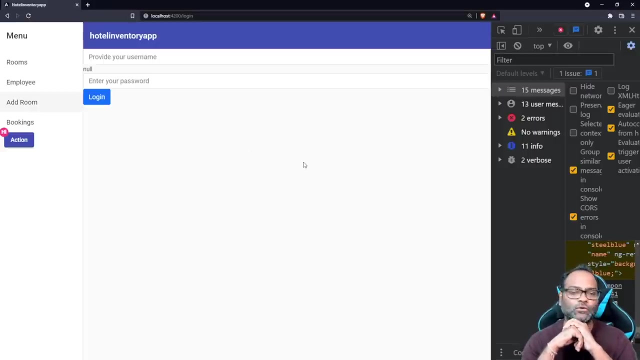 on employee route, i think- and then we got kicked out and there was an empty page. we will see how we can actually handle that scenario as well, but let's do first thing first. so what we need to do here is we want to actually write the code. sorry, we want to write the code. so once you are logged, 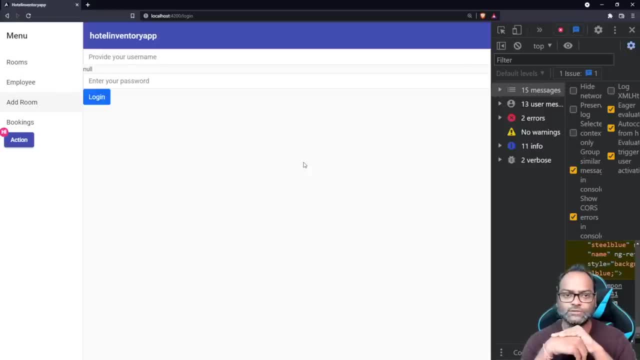 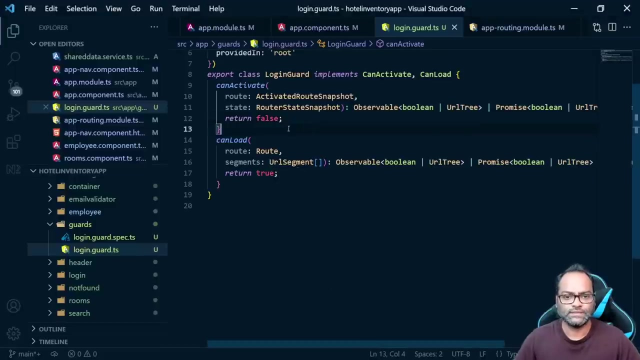 in and we- uh, or the end user is logged in and it's a valid user, that particular user should be able to access the routes so we can redirect to wherever we want to. for example, let's say, we will redirect to brooms, right, let's see, let's put that logic first. so in login, 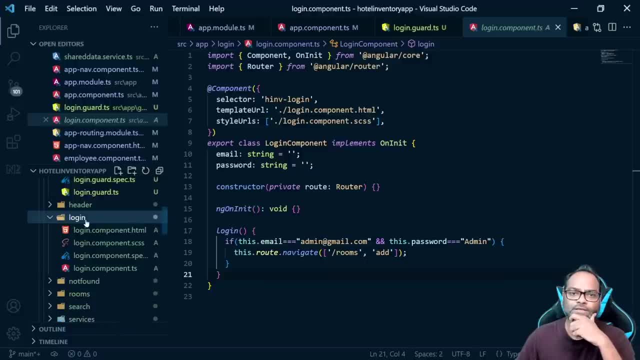 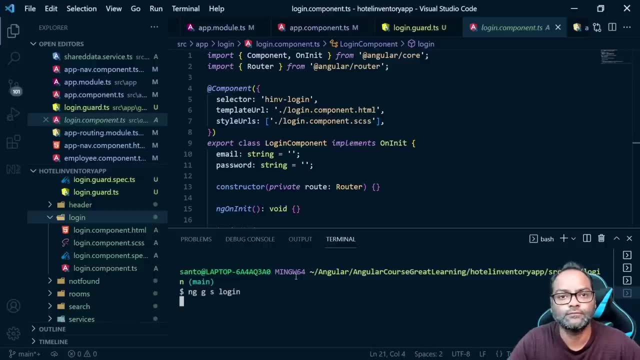 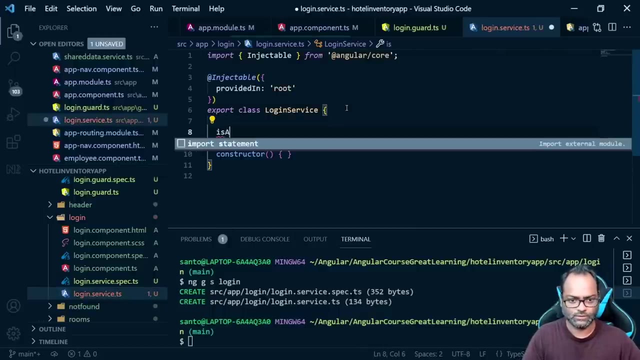 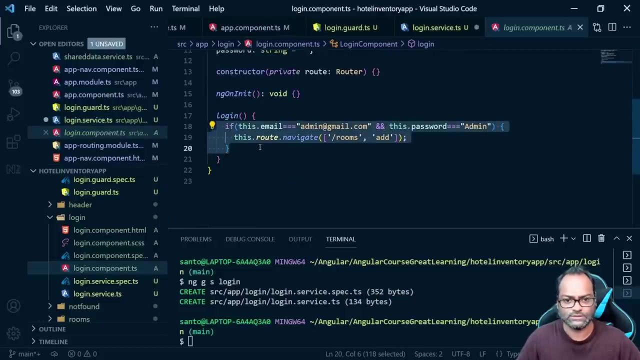 uh, what we will do is we'll create another service. i'll call this service as login service, and here i am going to put a flag which says is logged in, and we just type of boolean and false, and then i am going to put a method- login- where we will just copy the logic which we have already available. so i'll say this: 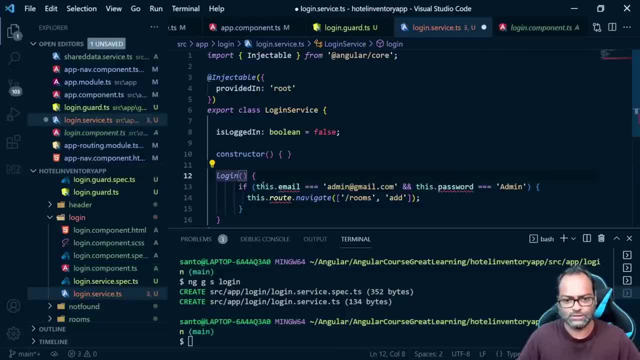 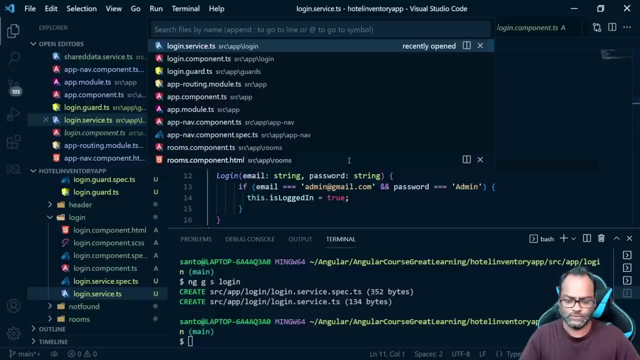 is uh, email and password. so i'll say email it's a string, and password, which is also string. but rather than doing navigate here, right, so we'll just keep the navigation part here and say: this shot is logged in is equals to true. so i'm just setting up the flag that, okay. uh, this particular user is logged in now. 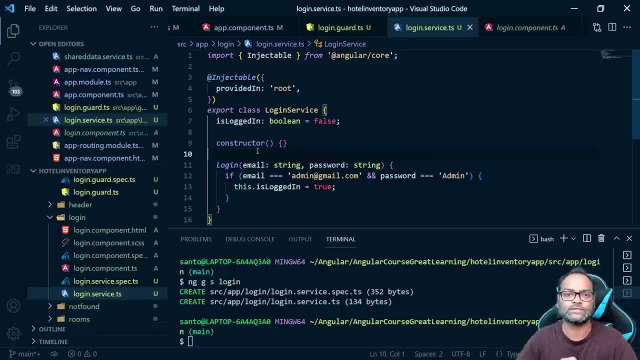 and as this is a singleton instance, everyone using this particular service will get the latest value for is logged in. you can do it in multiple way. do you want to use uh some behavior subject? go ahead and do that, but let's try to keep it boolean. uh, as of now. 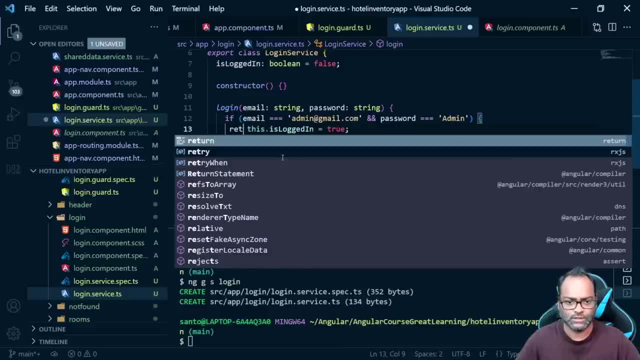 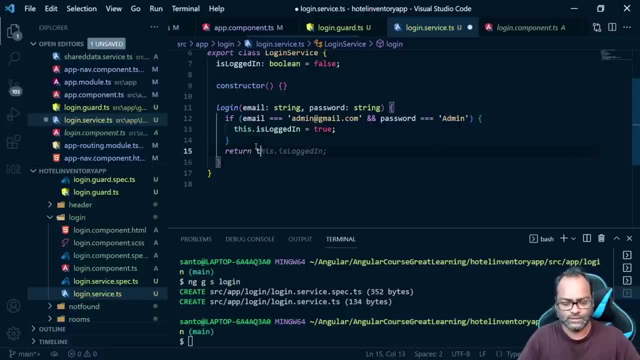 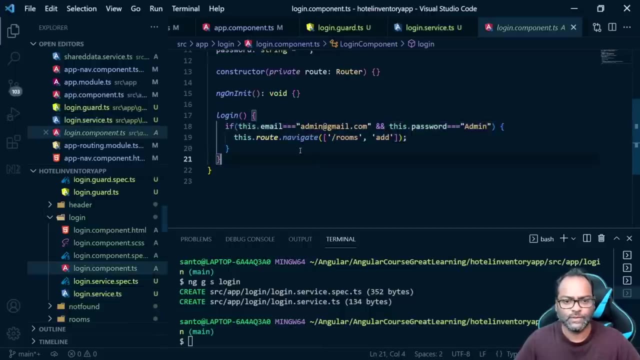 and if this is, uh, not logged in or we can just do something like this, right, so if let this and return this dot is logged in. so if it is not true, of course it will return the default value, which is false. and now let's go back to our login code and here say: private login service. 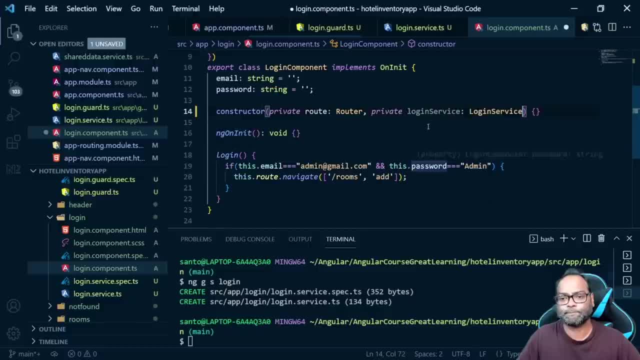 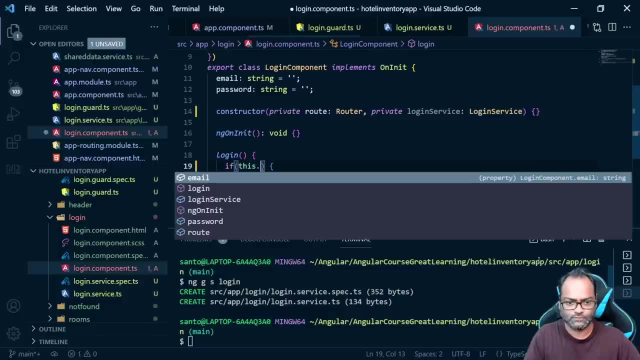 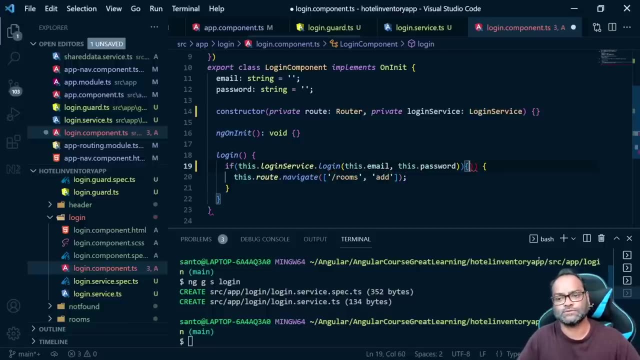 which is type of login service, and we will just check if this dot login service dot login and we will pass this dot email and this password. let's see if there are extra. so if this is true, we should be able to navigate to rooms. slash ad, let's try to. 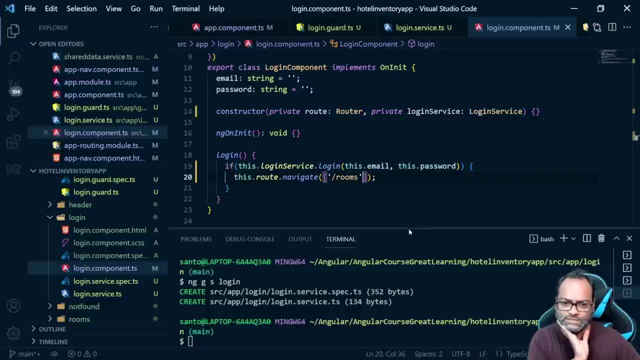 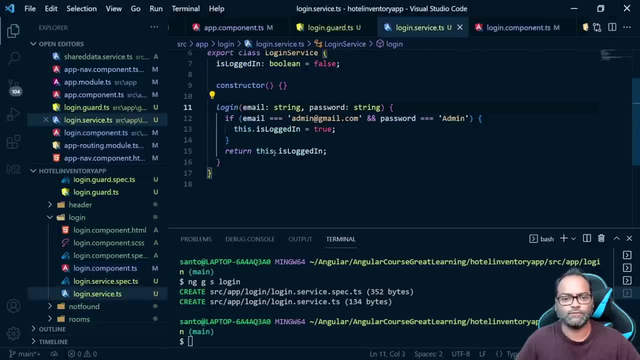 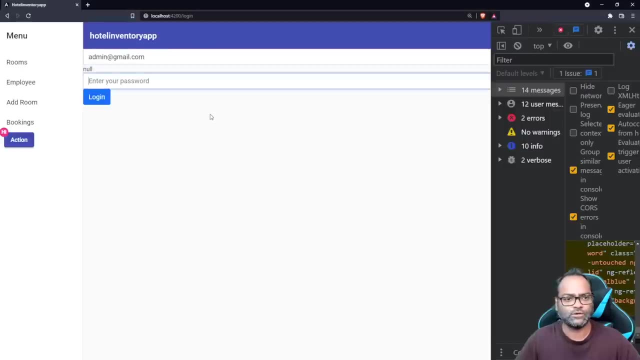 go back, go to rooms, right. we don't want to go to room, slash ad so, but still it will not work, right? so let's try that out. there isn't being. we have not made changes to our guard. are guard still returns false? so i'll say: this is admin at gmailcom and this is. 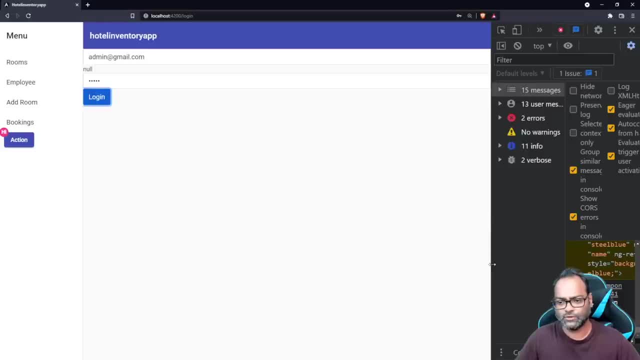 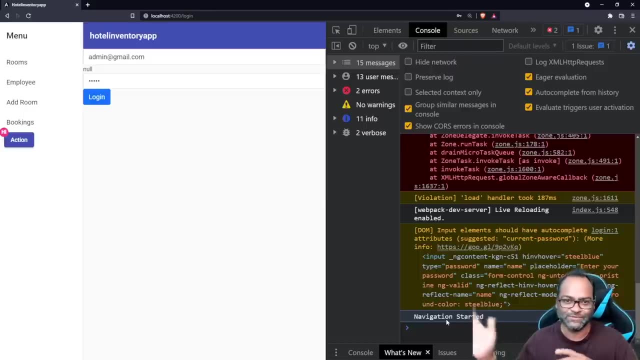 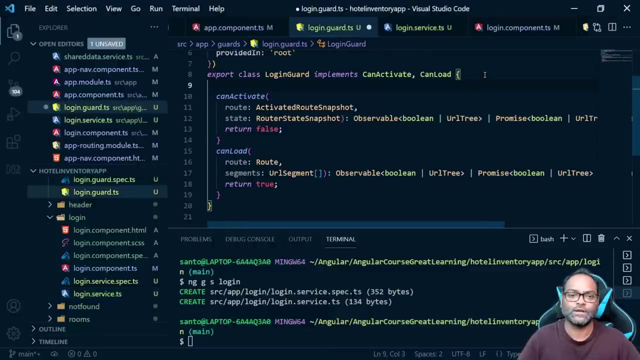 admin right, so nothing works. you can see here: navigation started, but uh, there was a guard. if it said: okay, you're not supposed to come here, just go back, go back. and that's where we will just write the code to our card. now how you can use login service here. 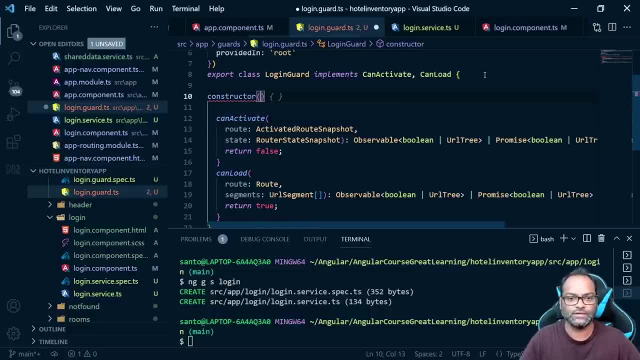 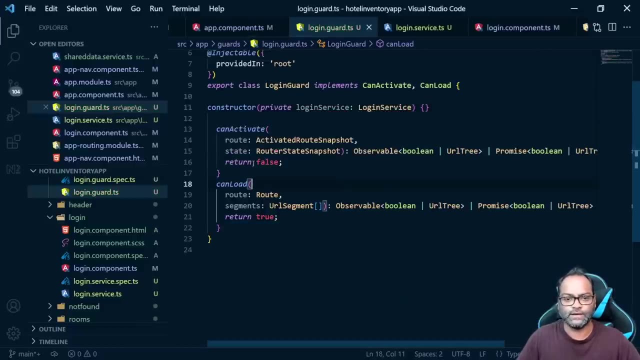 so remember, this is a service, right, so it also has a constructor. and then you can say private login service, which is type of login service. so now we have access to login service here. let me just close this and, rather than returning false, what i can do is return this dot. 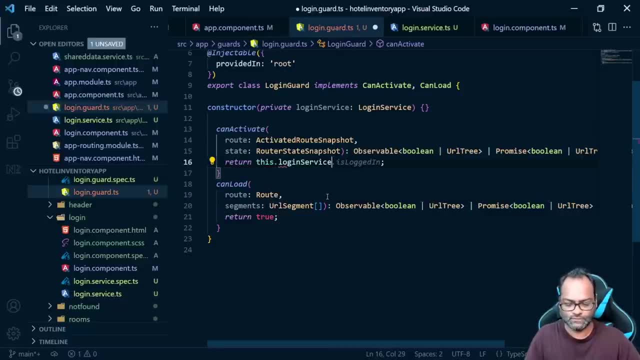 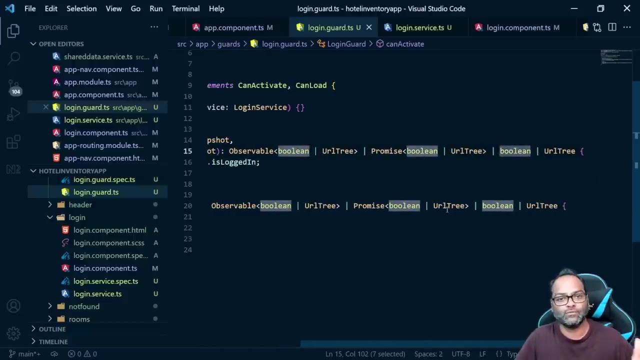 login service dot is logged in, so remember you. uh, it can be observable as well, because it can return observable or it can return a url tree. it can also return a promise which we are not using anymore, and also it can return a boolean which we are using right now. it's a boolean value. 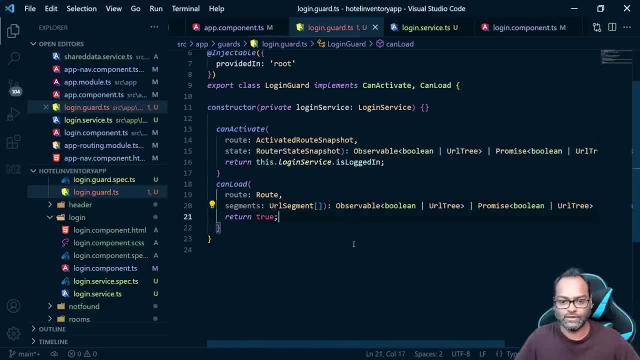 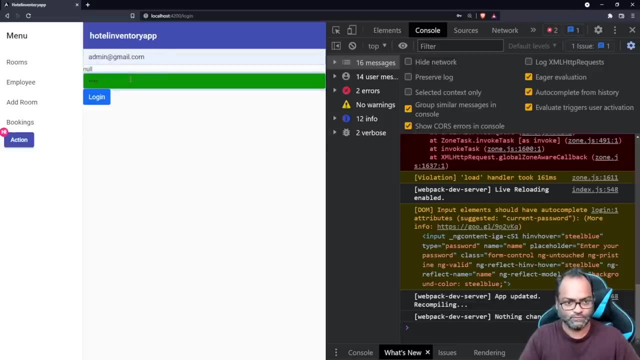 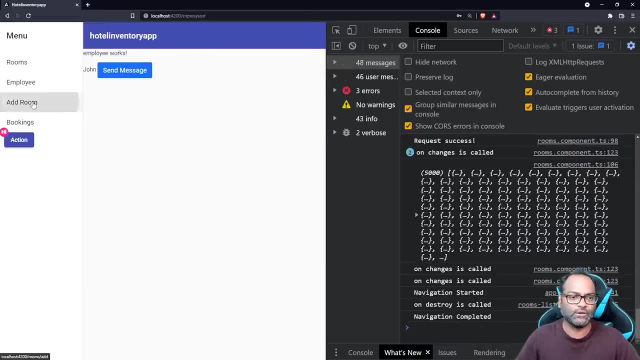 so now let's go ahead and verify the functionality. so i'll say, okay, this is admin, and password is admin, and let's click. and here it is. we are on rooms page. let's click on employee, let's click on add room and everything works fine, right. so because now your guard is saying: okay, i checked. 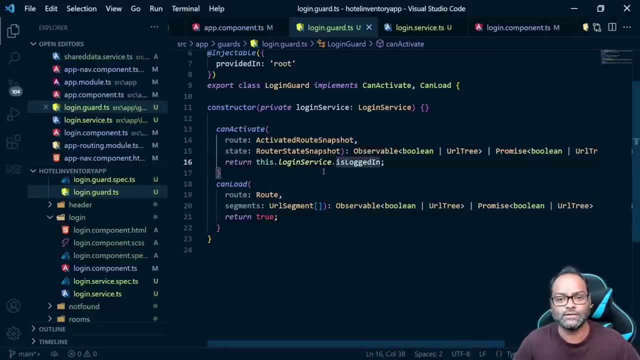 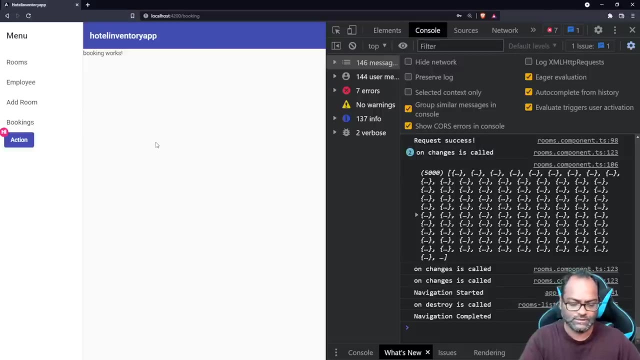 you, you don't have here. let's just go go into the bank. and, similarly, here, our login service is saying: yes, you are logged in, just go ahead and enter and access the urls you want to. so this is, uh, one way, uh, but let's try to do one thing: let's refresh this page. remember, now it's a blank page. we are not even on login. 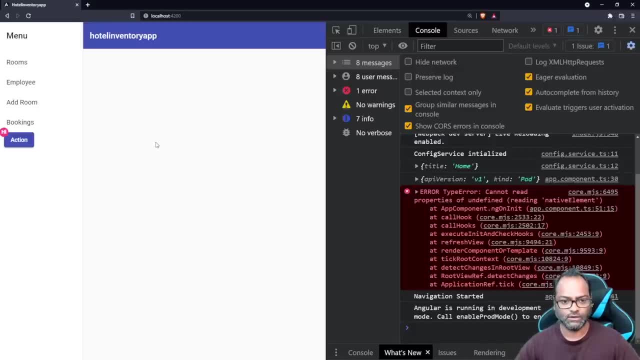 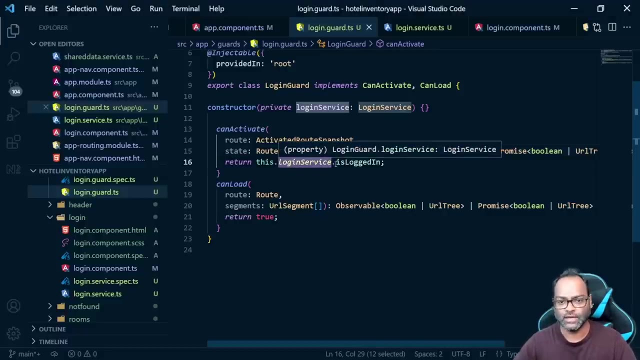 page. the reason being: once we refresh, of course, you lose the state of your application. in that case you be. your logged in state becomes false. but your guard does not know where to redirect to you. so it says: okay, i'm not sure where you uh, you want to redirect to you because you have already passed. you have already uh. 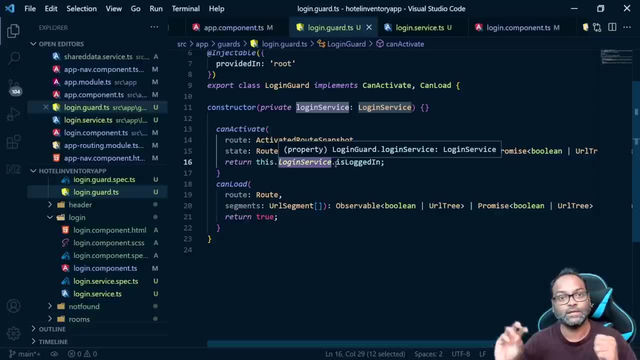 you are already passed the login, uh, sorry, the routes right. so you, uh, you have already checked the routes and you failed the what guards. you failed the card state, or you failed you failed the guard. check now where to redirect to you. so this is where you can do something like this, so 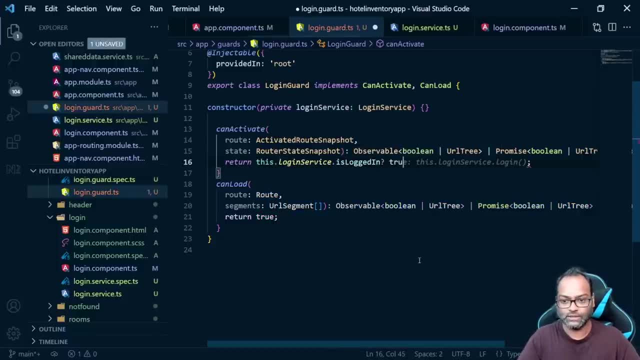 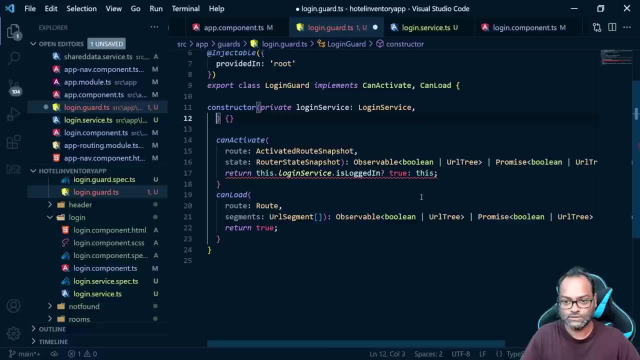 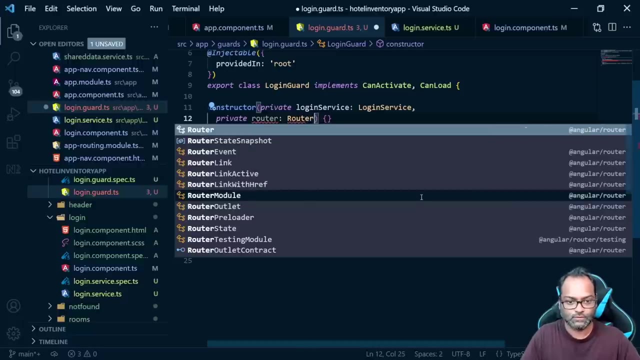 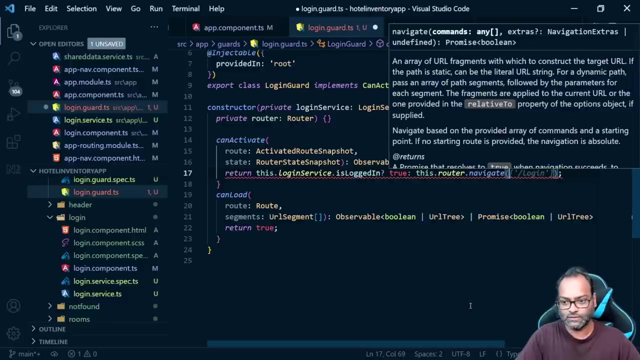 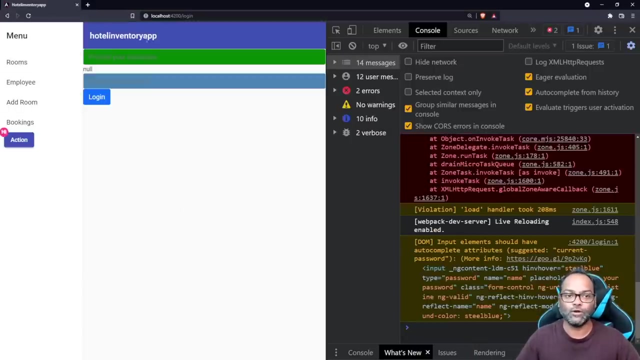 you can say return if logged in. then i can say, okay, return, true. or you can use the router service. so let's see, inject private router. so you can say this, dot router, dot navigate, and i can say just go ahead and navigate this user to login. let's see now, and here it is. so we are on login page. but you might be saying, okay, this. 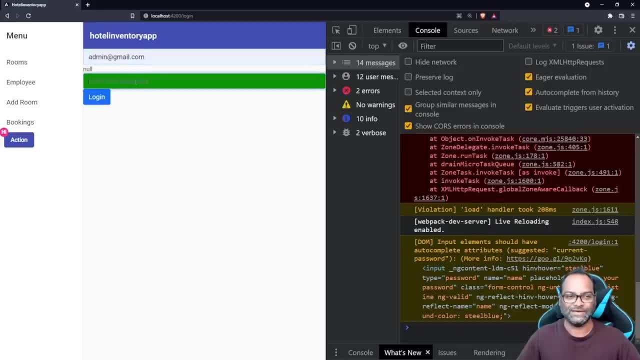 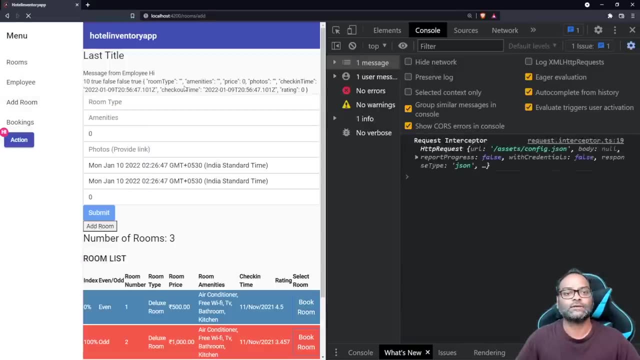 that was by default by us, you by your line. i'm not let me show you, so let's go ahead and say login and same thing, we will refresh and we are on login, so we fix that particular issue as well. so this is from: can activate card. 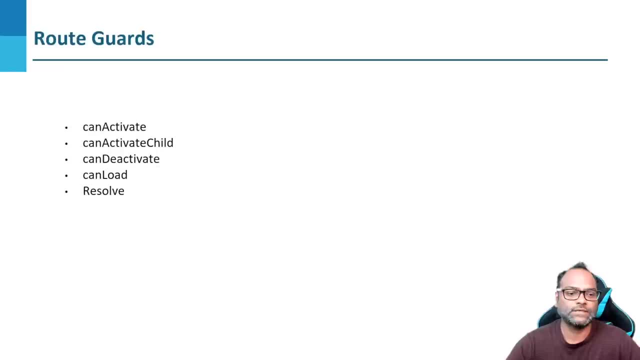 let's go back. uh, sorry now. now let's go ahead and discuss about connect with child. so it has something to do with child, as it says, and lucky, luckily for us, we have already seen some example how you can use the children property in your route. right, so we did it for rooms. 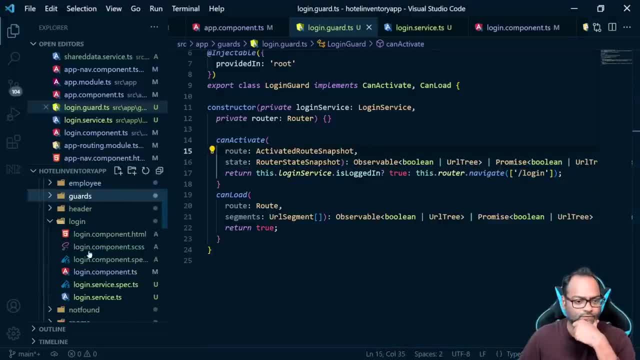 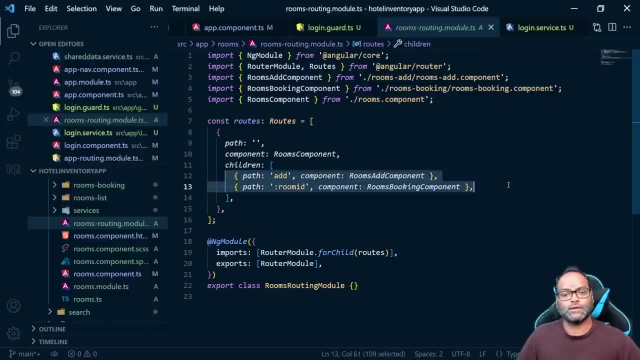 let's go back to the code. so here, uh, we have rooms, and then let's go to the routing and we have these two paths. so now, what we want to apply is we want to say, in case this logged in user is admin, i should be able to access children. otherwise, i should not be able to access children. 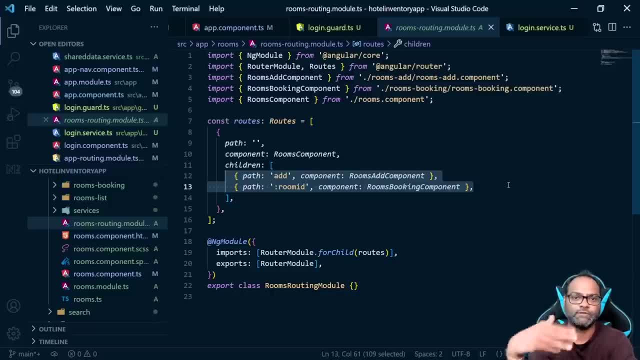 possible, right, as i said, i mean, even in banks. you can have a card. who can? who is responsible for checking what kind of role someone has? who is trying to access the, this particular logger locker? if you are a teller, of course you should. you, you can get the access. 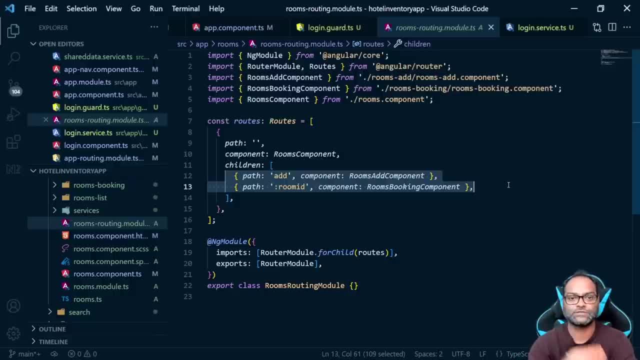 if you have, uh, if you are a user, you should get the access to the locker. but if you are someone who is not authorized to access the logger, you can get into the bank. so you pass the can activate guard, but you should not be able to enter into the locker room. that's what we are supposed to do here. 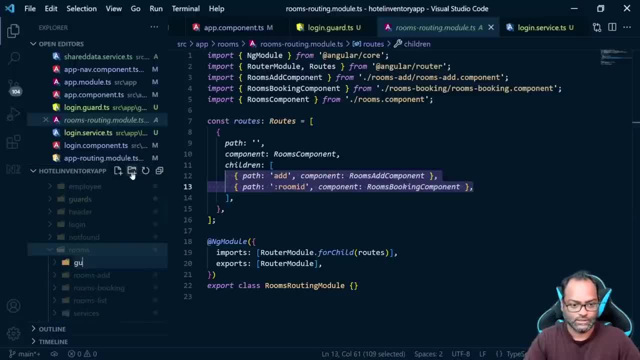 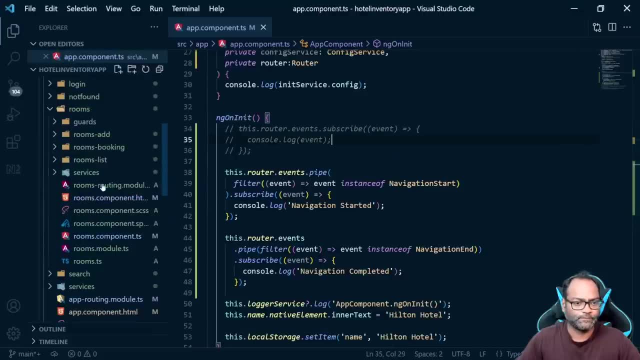 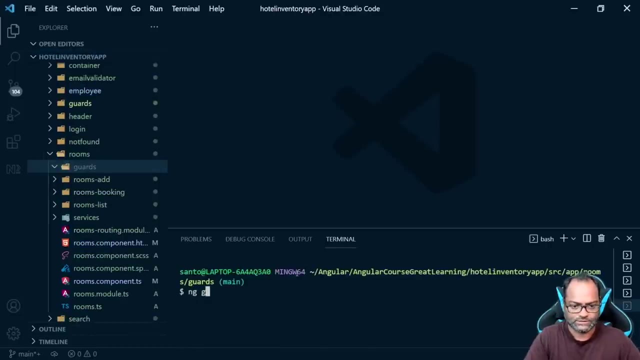 so here we will be creating another folder. we'll call it as cards, and this is related to rooms, so i'll just close others here and let's close this as well, because there were too many files which were open, and let's go to integrated terminal and gg. 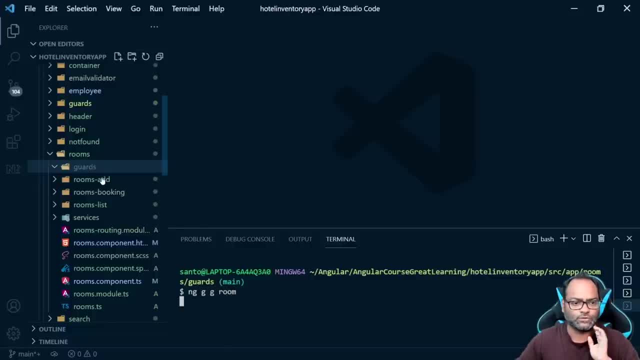 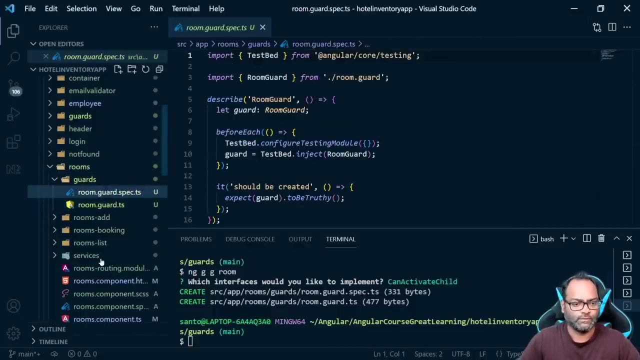 g and i'll say this is room guard, it is related to room. so in case in future we want to add more, we can. and the only card which we want here is: we want can activate child, and that's it right now. it's true, but let's go ahead and apply this card, so here you can say: can activate child again. 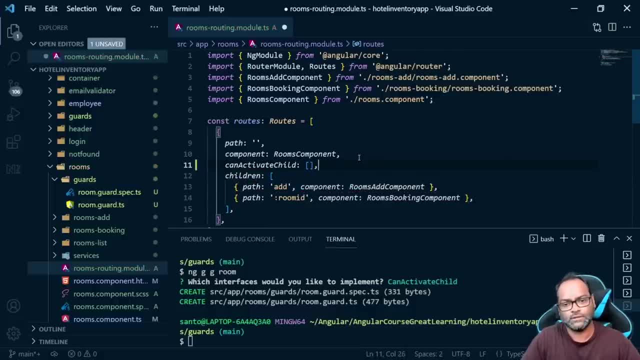 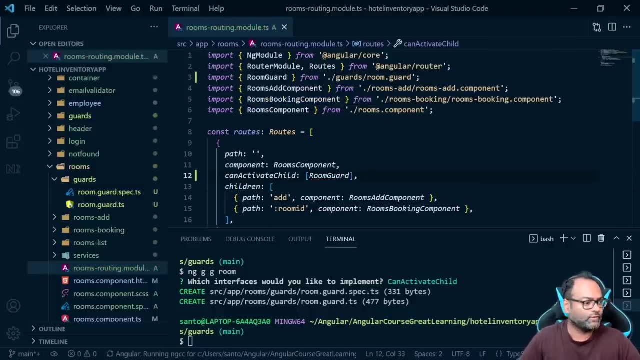 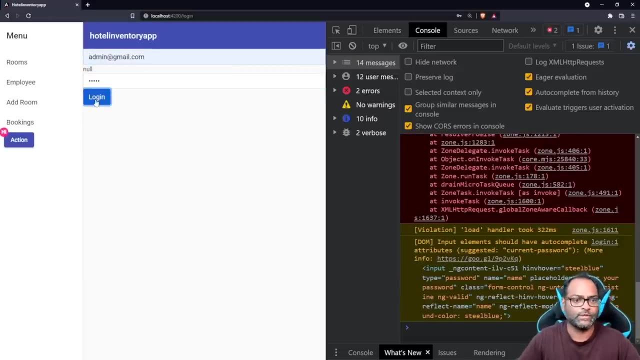 this is an array, so you can have a number of cards applied here and you can say room card, right, so everything great so far and we should be able to access once we are locked in. so i'll say: this is admin, admin, and we should be able to access rooms and add rooms. you should be. 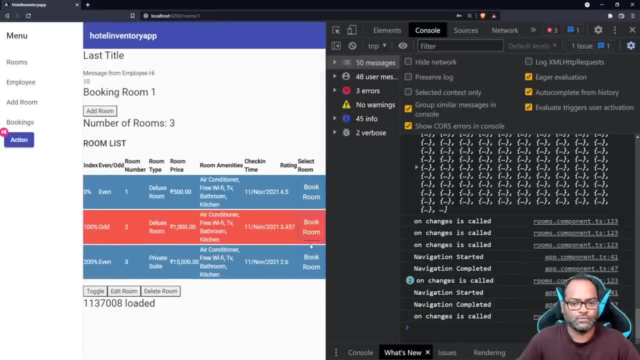 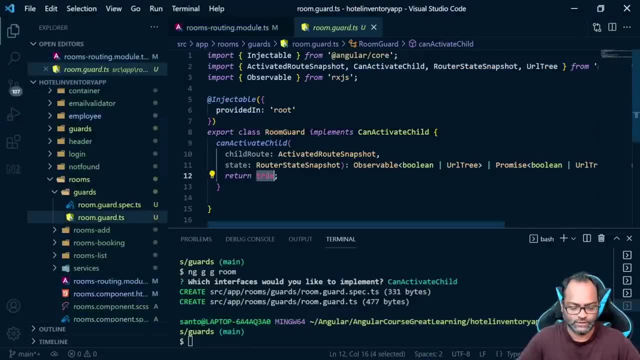 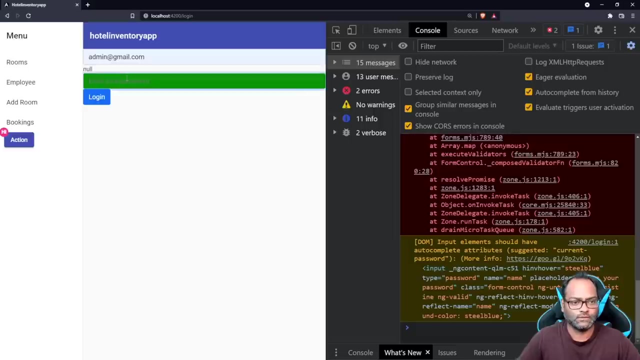 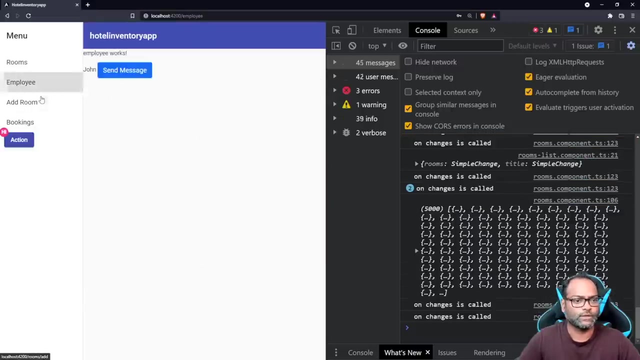 able to access book room and works fine. now let's break it. so to break it we have to say return false. let's provide admin, admin and hmm, click on employee, click on rooms- add room- now we don't have access. click on book room: we don't. 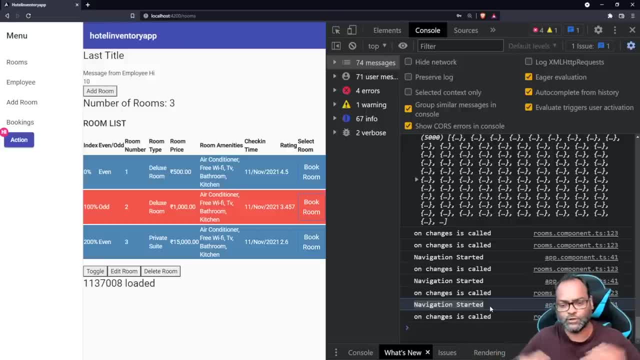 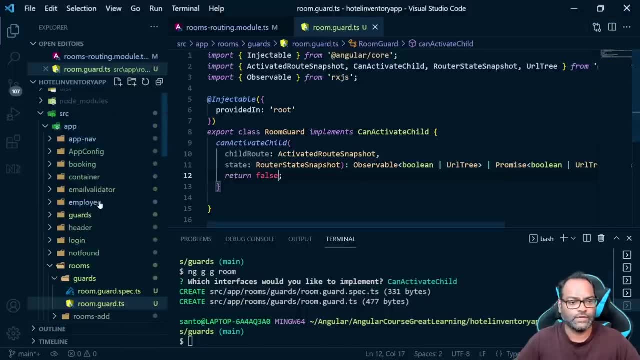 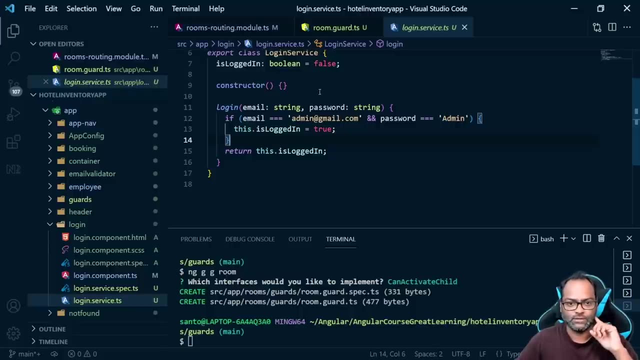 have access and it says navigation started but it never ended because because, of course, the guards kicked us out. let's now fix it so we can go to login. and now we are supposed to have two types of login. so one is user logged in a user login and one is admin. so i'll just add, i'll say this is is. 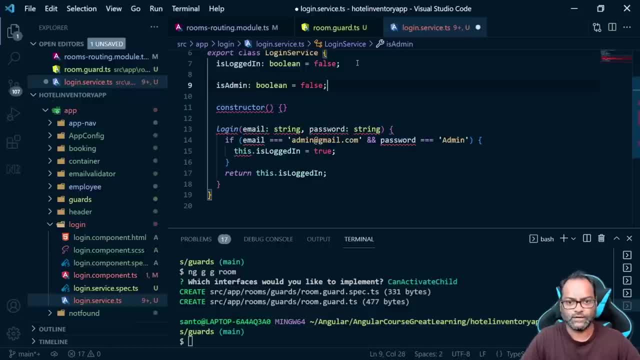 admin and which is boolean and which is false by default, and if someone uses this, so i'll say this is admin, which is true, and i'll say else, or sorry, not else. if else, you can just use it right. yeah, i'll say this is user. i can say: okay, this is logged in, is true now, but is admin is false. 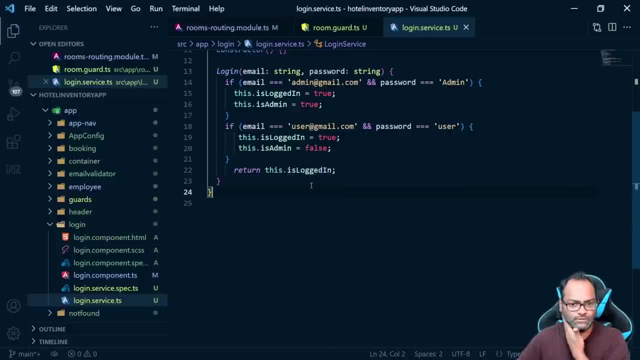 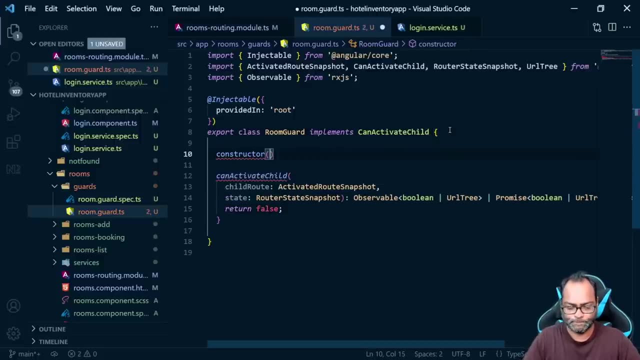 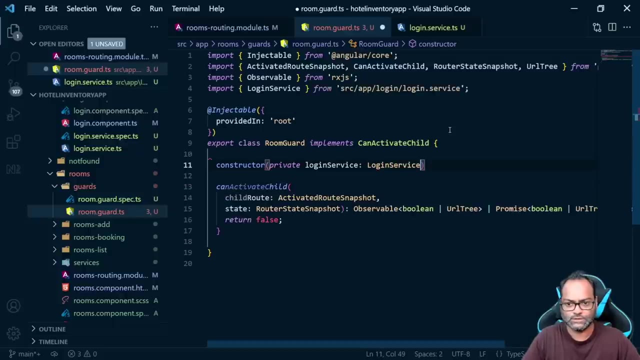 so now my login service knows who is admin, who is not. let's go ahead and use this into our guard so we can use private login service, straight up login service. and then here i can say: if written, this dot login service dot is admin. so if this is true, written, that's it. 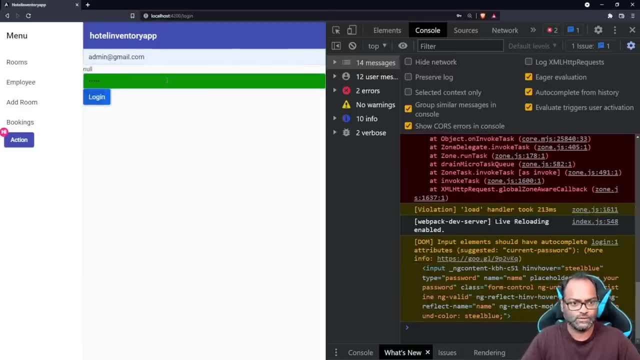 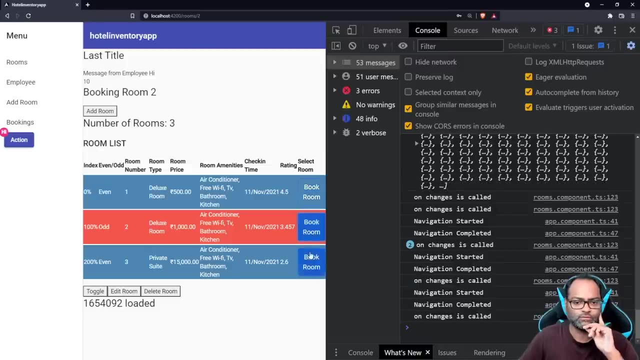 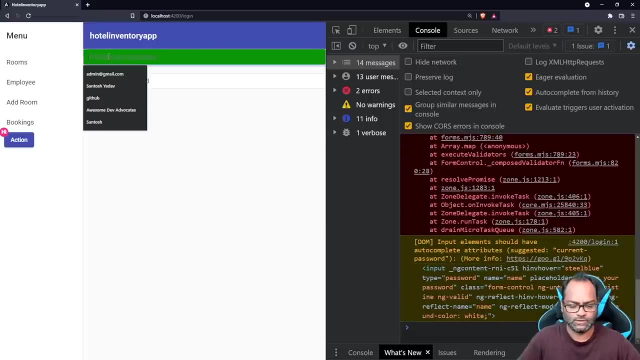 in case you want to add some extra check, go ahead and do that. let's figure out admin first. add room: yes, works. select room: select book room: works. let's refresh this page so we will go back to login now and now you will. you will use user and create gmailcom and we will use user right and let's click on add room. we 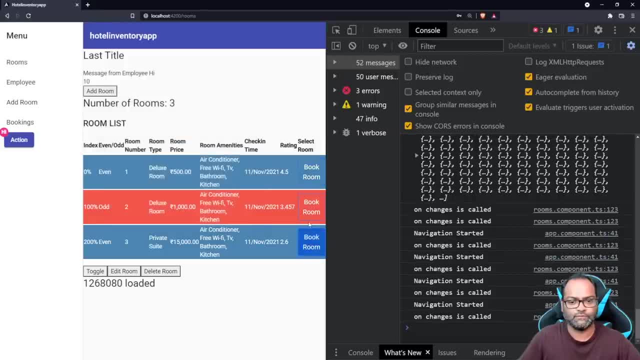 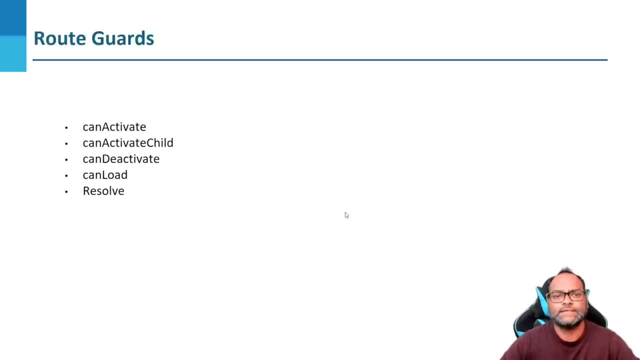 don't have access to it, select books, and we don't have access to it either. so this is how you can prevent the access to child rubs. this card we are going to talk about is not can deactivate, but we'll talk about can load and then we'll come back to can deactivate and resolve card. 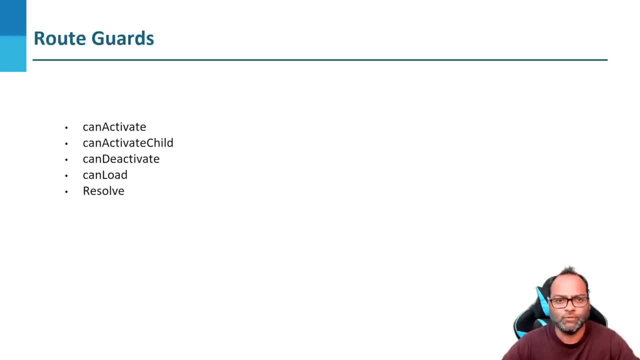 so why i mean in can deactivate? we need a form. so we will go to the another topic, which is the active form which is pending right now, and we'll create a form and then we'll come back to can deactivate. activate, because the scenario is related and i don't want to skip that. let's see. can load. 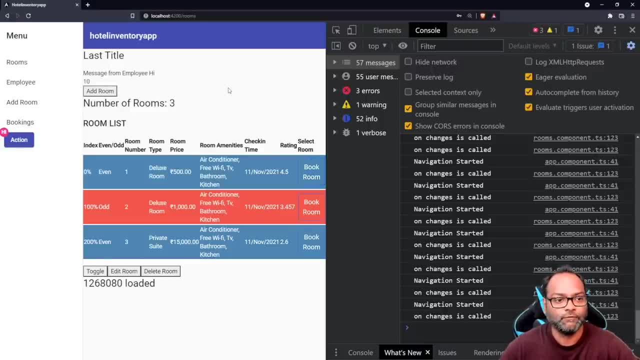 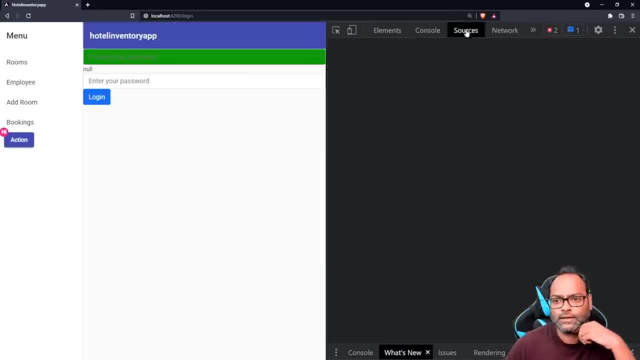 we already have an issue which is related to where we can apply, can load, so let's go ahead and refresh this page so we will be redirected to login and let's go to sources and let's see what are, what is the code which is loaded right now so you can see. you can go to apps and 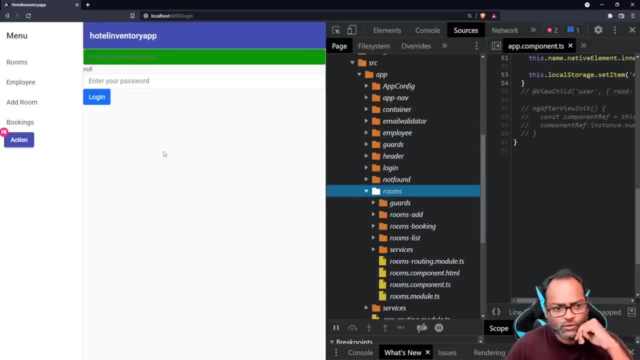 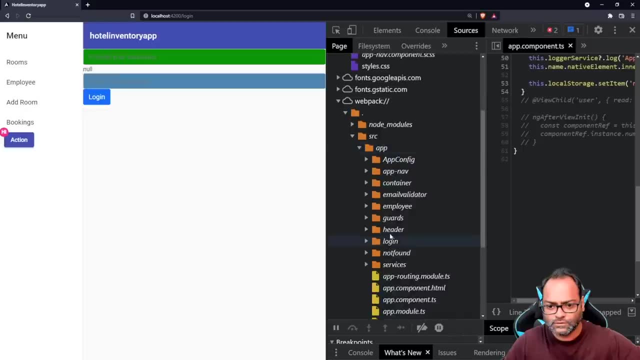 rooms module. what's this possible? let me just refresh again. so, yeah, rooms is gone, right. so we don't have rooms available here, which is okay, right. i mean, we said we already tested this. then you might be wondering why i'm talking about talking about this rooms again, which is lazy loaded. we know that it. 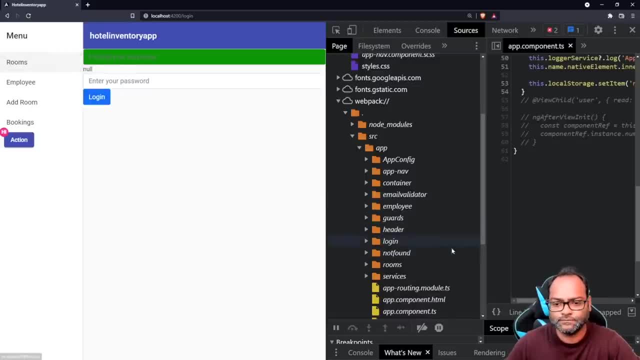 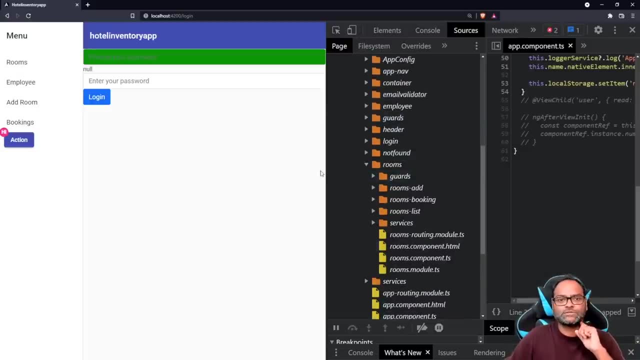 is not supposed to be loaded. let's go ahead and click on rooms so this rooms is loaded. are we redirected to rooms? the answer is no, but still have access to this particular route, the reason being we are not redirected because of can activate card. so we are not able to activate this particular route, but it is loading the code because it doesn't know. 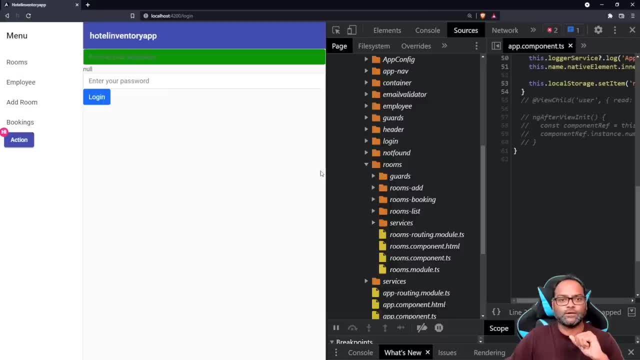 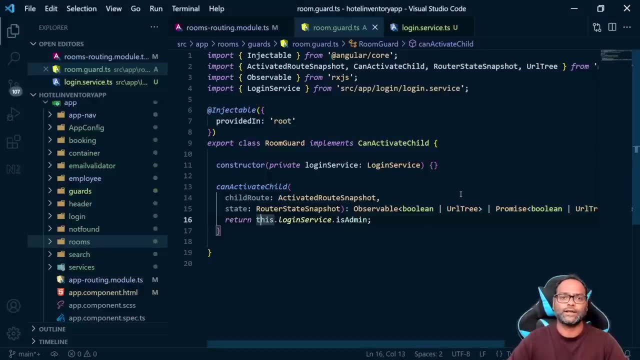 what to do in case i'm not authorized to access this particular route. this is where can load this is. this is where can load router card comes into the picture. so this is where the can load card comes into the picture. so it is itself say it is saying that can i load this particular route? it is only applicable for lazy. 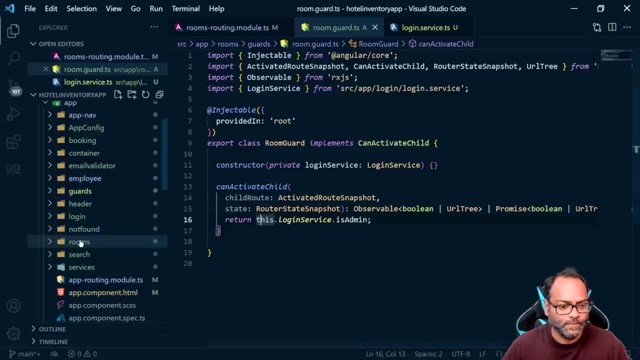 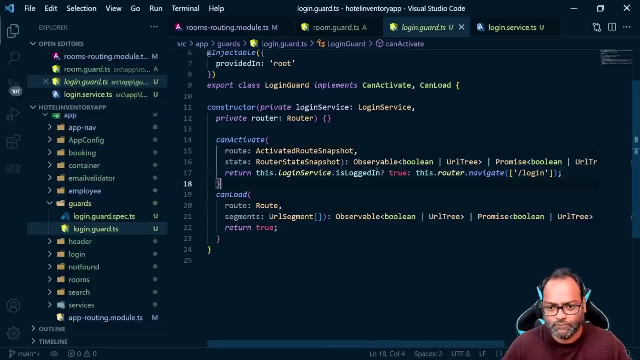 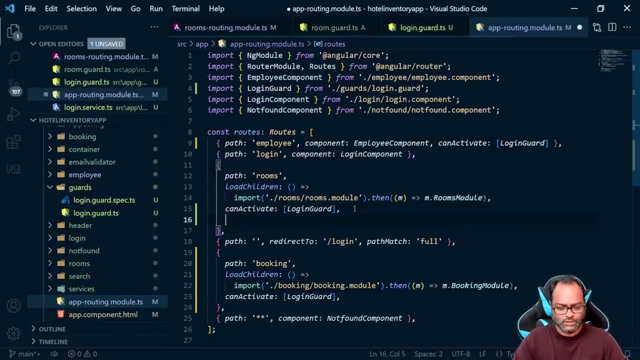 loaded route. remember this so i can apply this can load card. so i can just go to guards and i can apply this the same, apply the same. so i can just say: logged in, right, and let's apply the card here. so this is rooms. i can say it can. 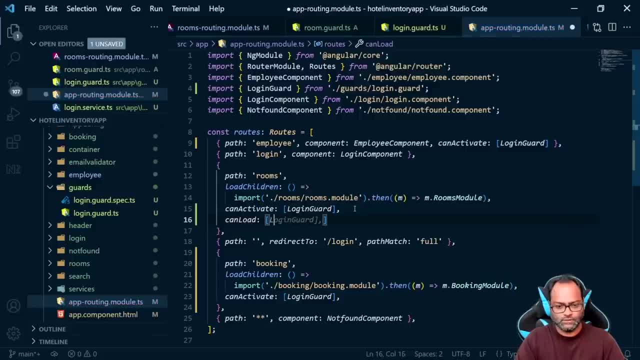 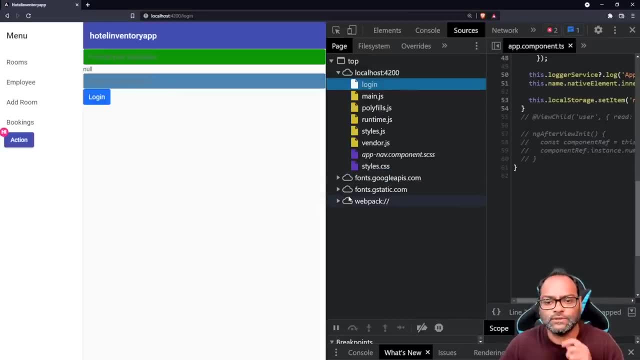 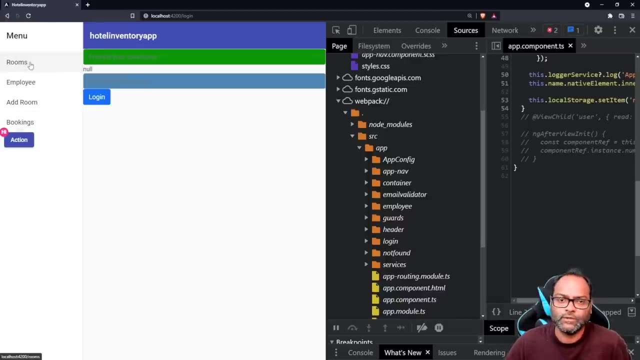 load and then i can pass the card and you might have a question again. i will come back to that point, but let's go ahead and verify this one. so i will go to webpack src app- rooms not available. let's click on rooms. and still not loaded. because now it knows though, okay in case, if i am not logged in, i'm 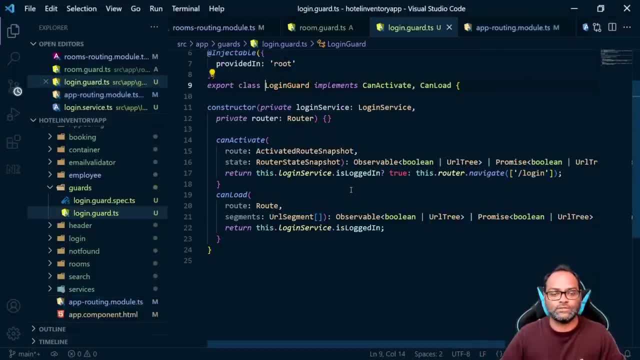 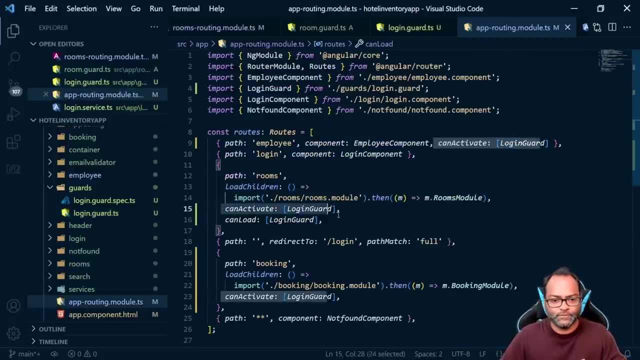 not supposed to do anything. i'm not supposed to allow access to this particular- sorry, i am not supposed to load this particular lazy loaded module. so that's what we are restricting here. now let's come back to this point, because you might be wondering that for can activate and can. 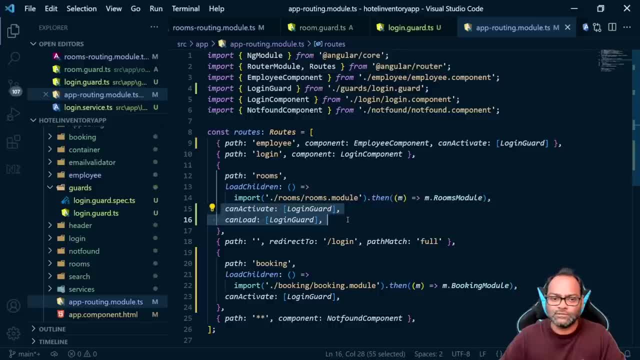 load both. i am applying login guard. i mean i can just go ahead and have uh, can activate child here as well and i can have. sorry, we don't have child, but in case we had right, so we can also apply um here. the reason, the reason they don't have child here is that they don't have the access to the. 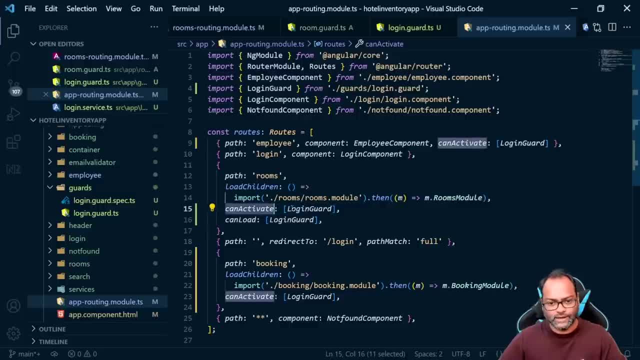 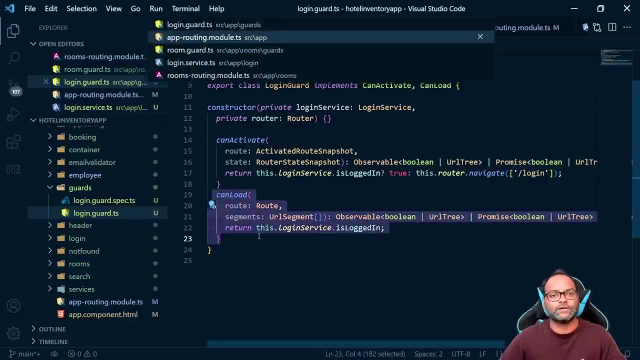 reason. the thing is, whenever it tries to actually apply or run particular guard, it checks for which property. so here though, even though we are passing login guard for both in this case, it knows that i have to go ahead and activate this can load function. in this case, it knows that i have to. 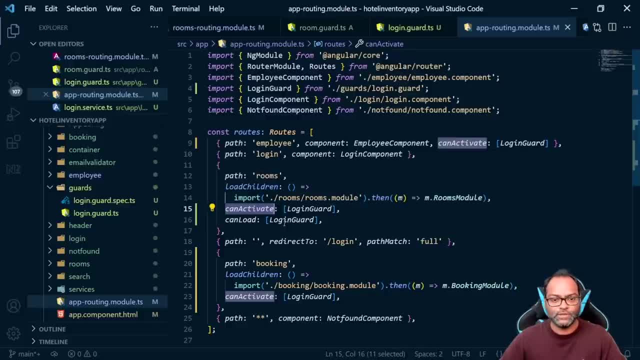 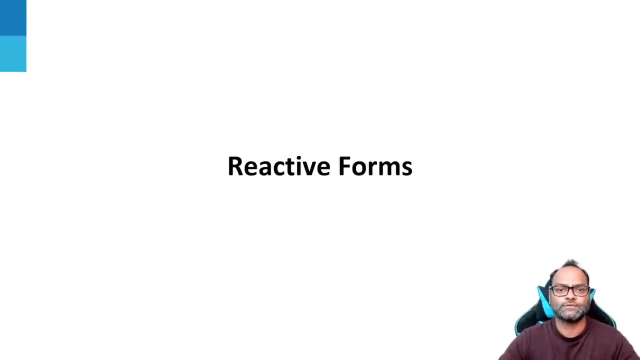 go ahead and implement: uh, so you call, can activate method, that's all. so that's absolutely fine. so don't get confused here, um that i have to go ahead and, uh, create multiple guards for multiple use cases, even though, even though the code is same, no, you don't have to. before we go ahead and explore, 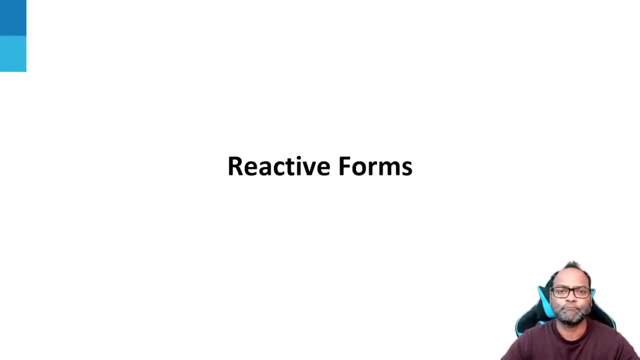 the other cloud guards which we had, we'll go ahead and create a form. so we already have something called booking which we want to create. so we want to create a booking form where users can book a room right, so, as an in someone who is working in that hotel, you will, you should be able to book a room. 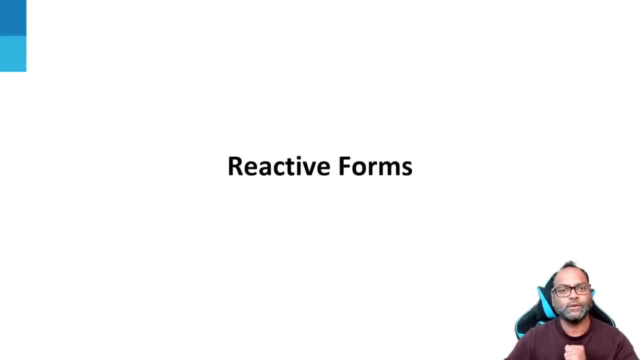 and that will be the form which will be created. so we will be using another approach called reactive forms. we already saw template driven form and here in reactive form as well. we will go through: uh, step, we'll do, step by step. we'll set up reactive form, then we'll talk about. 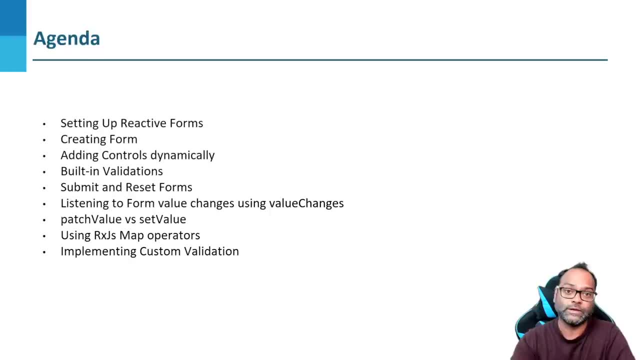 we'll- uh. we'll see how to create a form. then we'll also see how to create- uh- add controls dynamically. then we'll talk about the built-in validators. we'll talk about submit and reset form. we'll talk about how you can listen to the changes on a. 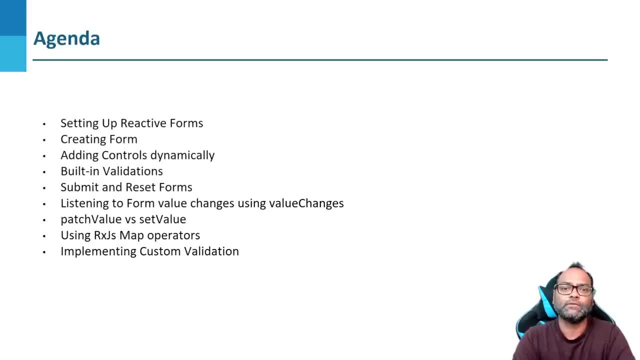 form, which will be, of course, using template driven form. we'll also talk about patch value, set value, which is really important. uh, important question in case you are giving an interview. we'll talk about few rxjs operators and then we'll also add a custom validation. so let's go ahead and 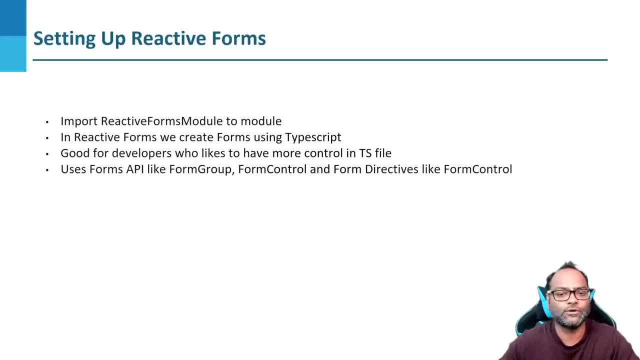 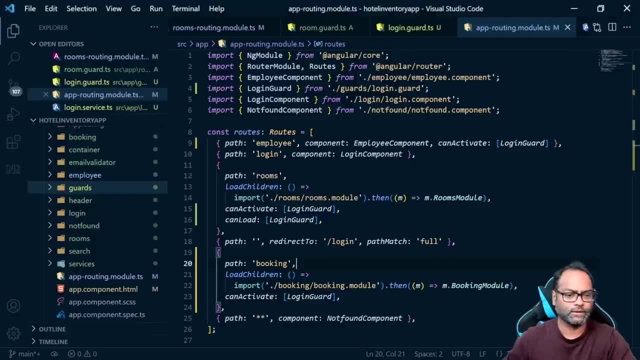 start with setting up your reactive form. the first thing which we need to do is we need to create or import a reactive forms module. so let's say, we want to create a new template, we want to create a new form, we will be doing it for booking and for booking we already have a module. separate module. 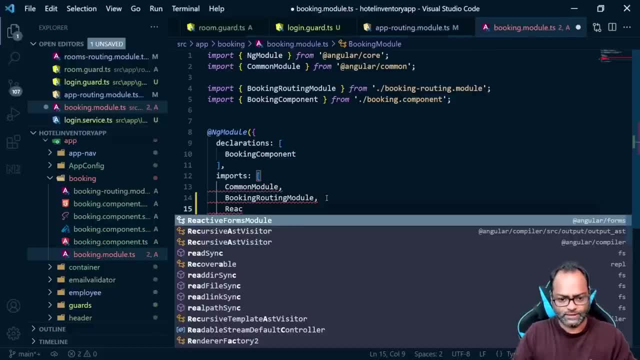 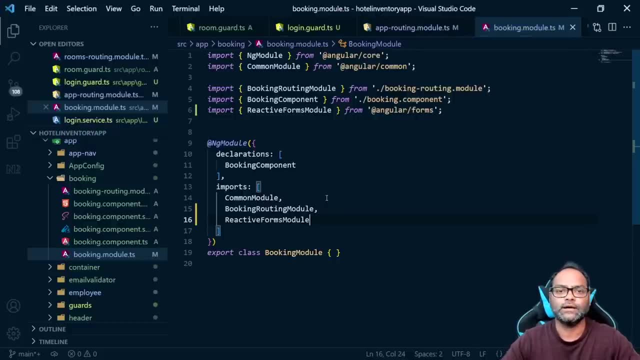 so what we will do is we will add a reactive forms module here and remember, in template driven form, what we saw is we created the in in template driven form. what we saw is we created the entire form using html, right in template driven form. you will see another approach. we will see that all the forms will be created using st, using typescript. 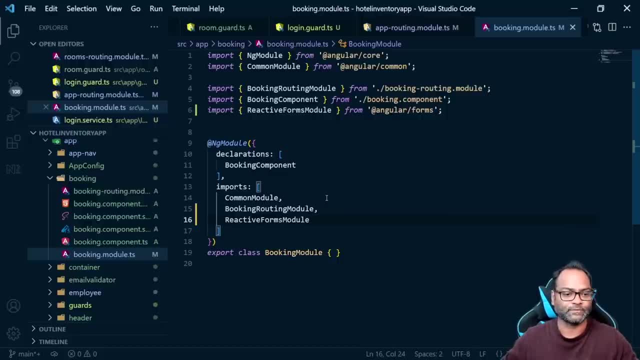 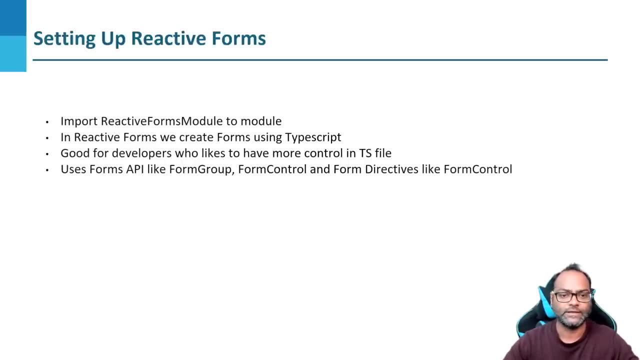 and we will just be rendering that those forms which is already created. so now, first step is done: reactive forms module added. now let's go ahead and see what else. so we'll create reactive form using typescript and this is a good approach in case you want to have like more control on. 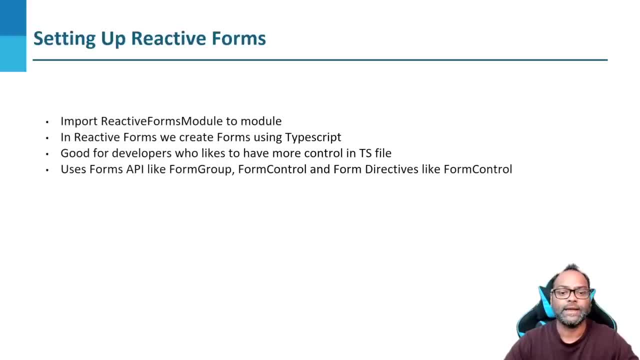 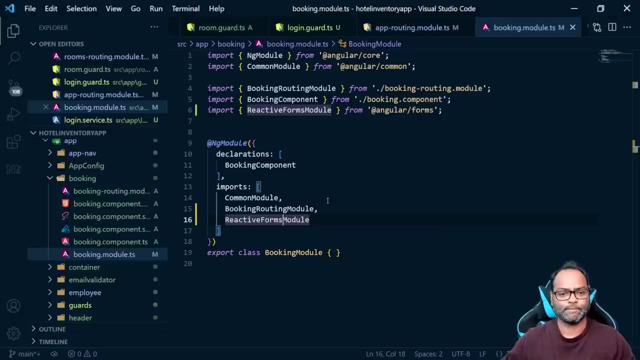 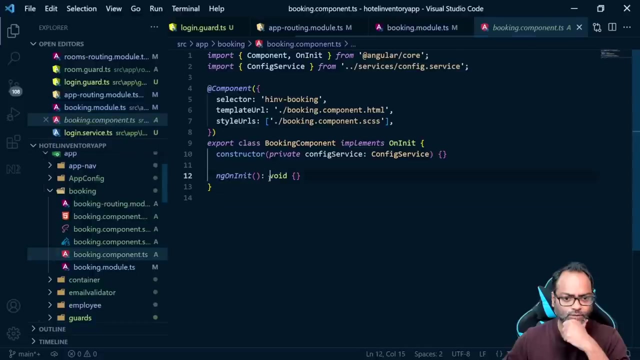 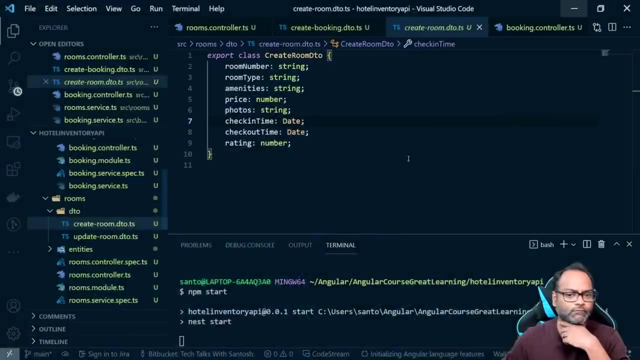 the typescript side of over of your form and, uh in case, uh, sorry, the apis are same. as i said, but you will be using something like form group, form control, form directives, uh, so let's go ahead and do that. so here. uh, let's first see how our form looks like. it means we have to have a model, so 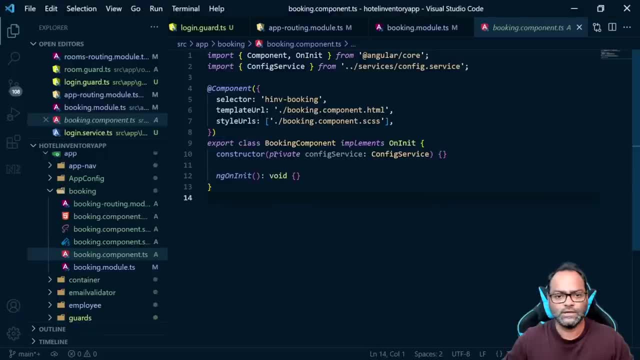 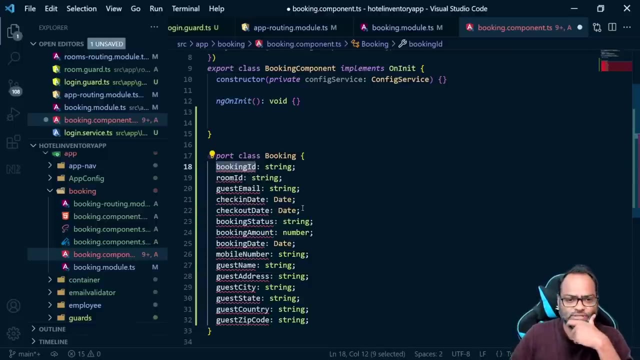 here i have created a model which will, which will show you how my how the form looks like, so let's paste it here. so we'll be having a booking id, which will be auto generated so we can remove this. we will have a room id, of course, because we will book a specific room. then we will have 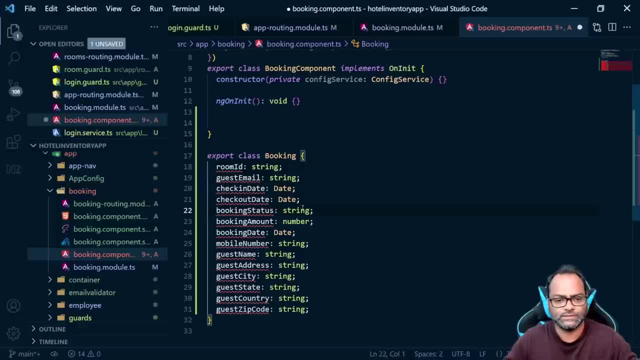 email. we will have check-in date, checkout date. we will have booking status, which will be generated- uh or we can send it. so booking amount, booking date. we will have a mobile number, guest name, guest address, city, state, country and zip code and we'll also have guest count. so type of number and, in case it is, number of guests are: 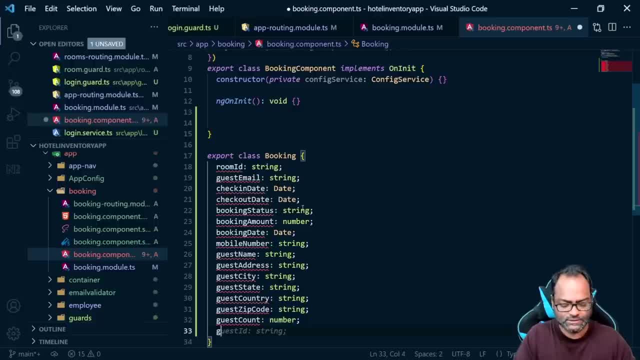 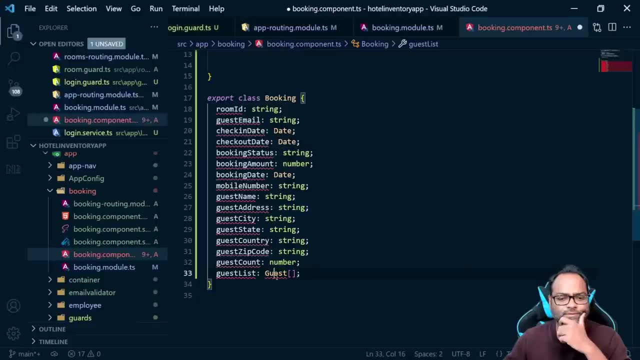 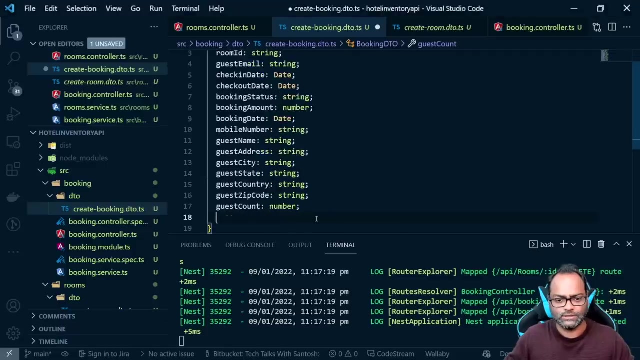 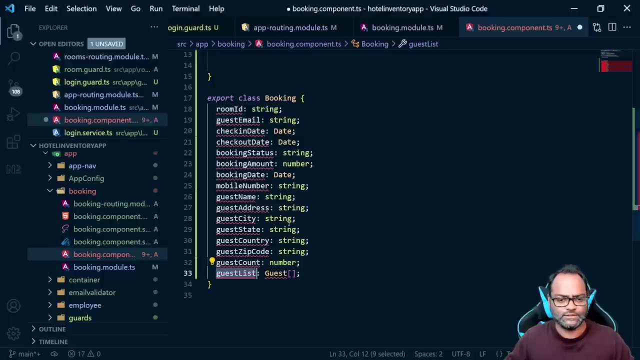 more than one, right? so we have to have that guest list so we can say: guest list and some random thing, right, some some random object. so let's go ahead and add. let me just add this into my back end, because i have not done that and it's a guest list which will be the array. okay, so i'm not creating an interface here, but 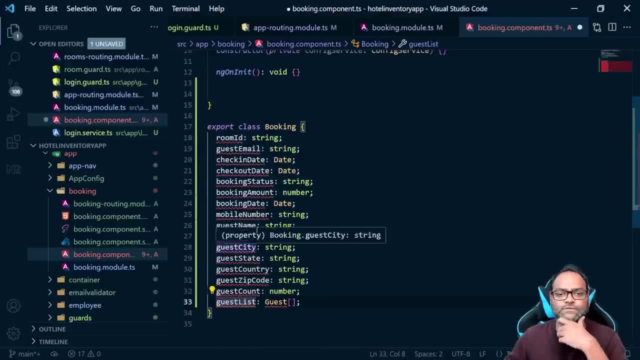 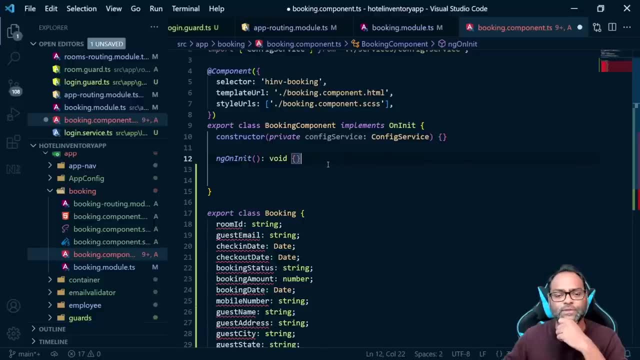 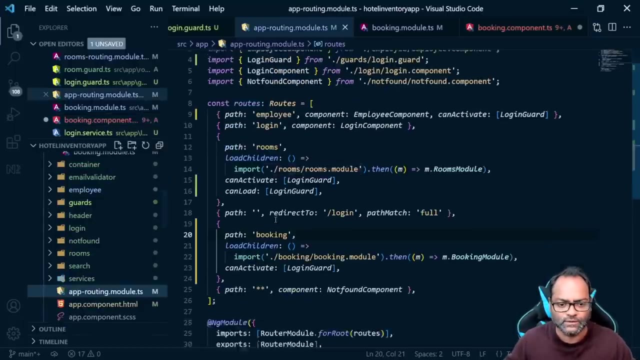 it's absolutely fine. but, yeah, i know this is these are the fields which we are supposed to have. so let's go ahead and see, uh, how we can create this form using reactive form. so the first thing which we need is we need, uh, the first thing which we'll do is we'll do one thing: i'll remove this connectivity card from here. 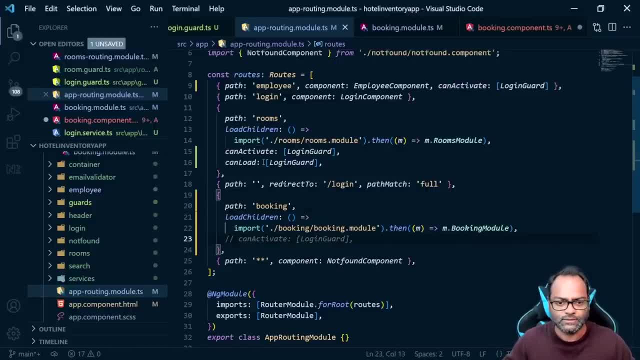 i don't want to actually log in every time, and let's do it here as well, and we'll put it back. the thing is: uh, here, i need this one here, so let's use this here. let it be, we can keep this and let's do it for booking. 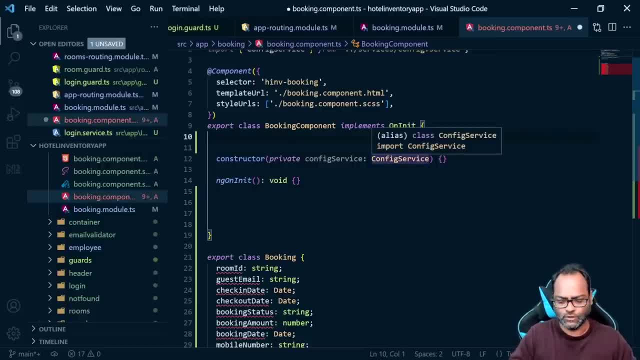 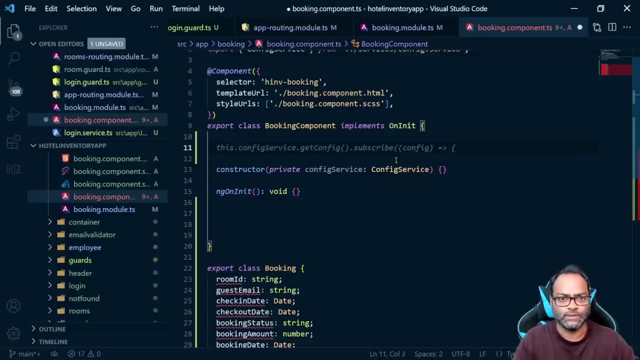 so, booking component. uh, the first thing which we need is we need a form. so how we'll create a form? so there is a class called form group where you can actually go ahead and add multiple controls. we will see some other variation as well. what in case if i don't want to actually have entire form? 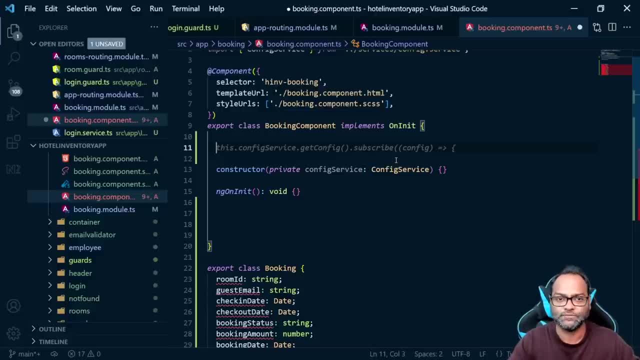 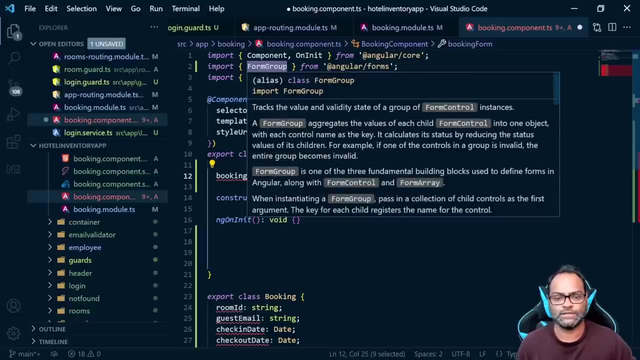 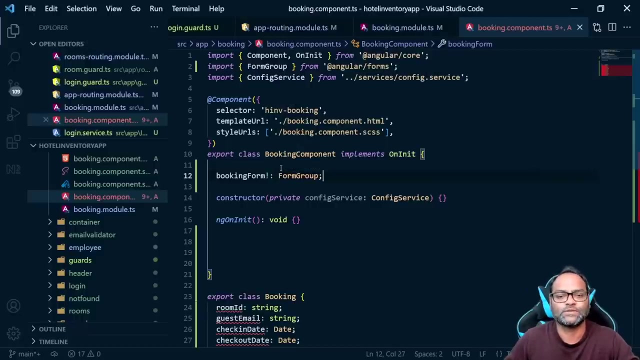 we need a single control. we'll see an example of search. i'll call this as booking form, which is type of form group. so this is the first class which we are using form group and we are saying, okay, this booking form, let's use this, so we don't have the 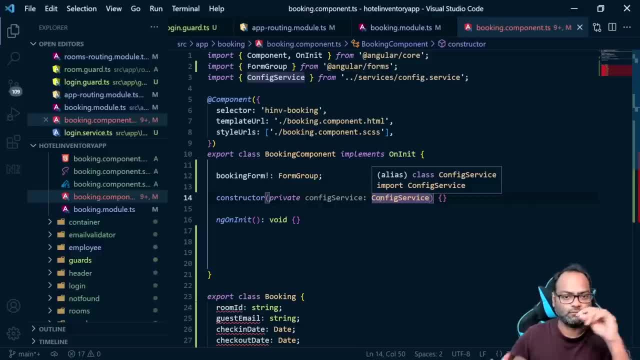 error available here and then we now we need we have, we got our form, so it's an empty form. what else you will do after you got your form? you will add controls. how you will add controls, so let's go ahead and see that. so there is a class called form builder. the name itself suggests that. okay. 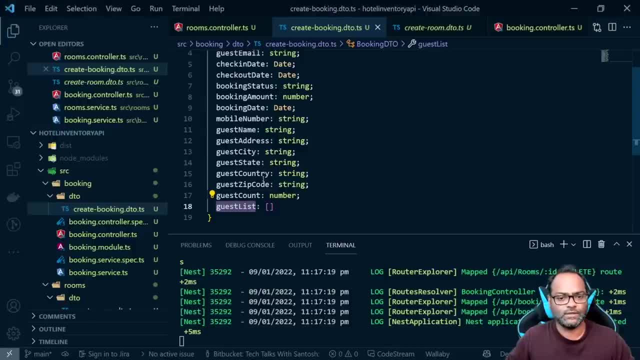 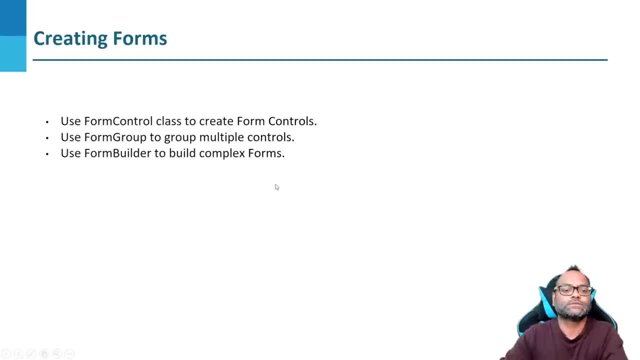 this is something which will be used to build the form. let's go back to our slides here. yeah, so, uh, we will go through form control later on. uh, for another example, but here, so we can use form group to group multiple forms or multiple controls, and we will be using form builder to build complex forms, so it can be used to add multiple controls. 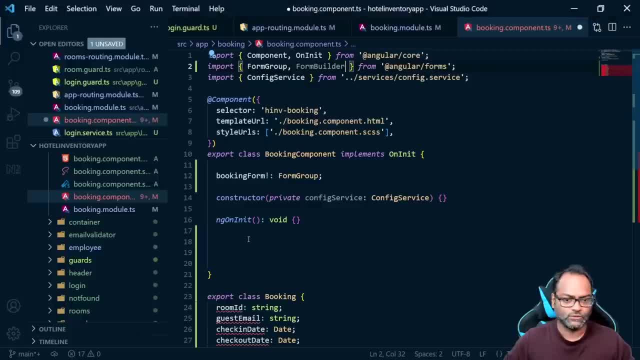 to that particular form. so now let's go ahead and do the step two. so we want to use form builder, so i will use: this is a service, remember. so form builder is a service, so we are injecting it. we'll say, okay, this form is form builder, and then we can say this: dot, uh, your booking form is equals. 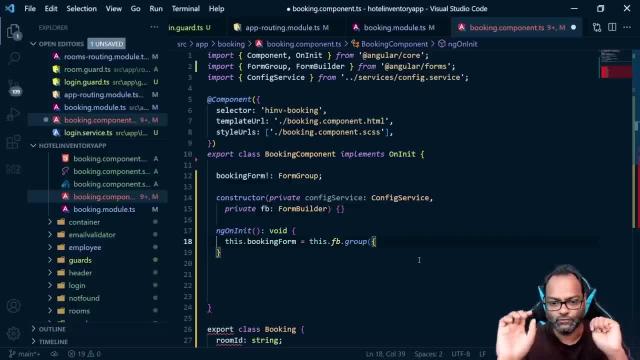 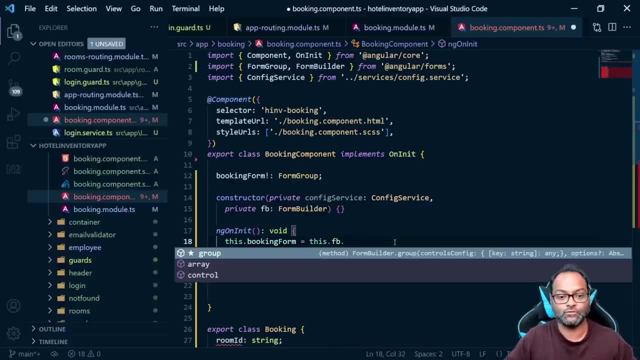 b dot group. we are grouping the form. there are multiple ways. we will talk about how we can create a control because this form builder allows us to add multiple things so you can see it says there is a group, which is my widely used. you can say: there is a star in front of it means it is. 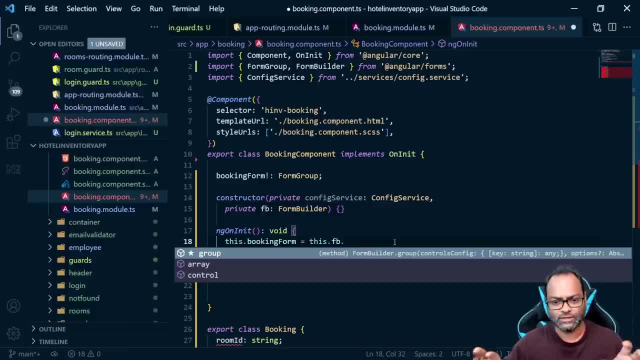 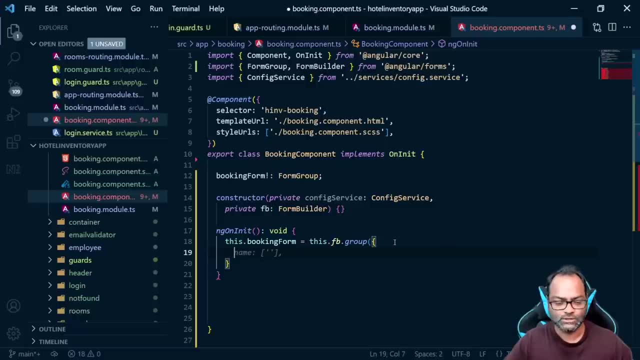 widely used. and then we have array and control. we'll see all the examples, don't worry about it. so right now we are saying, okay, there is a group and now in this form group, we can add multiple controls. so let's go ahead and add that. all despise. 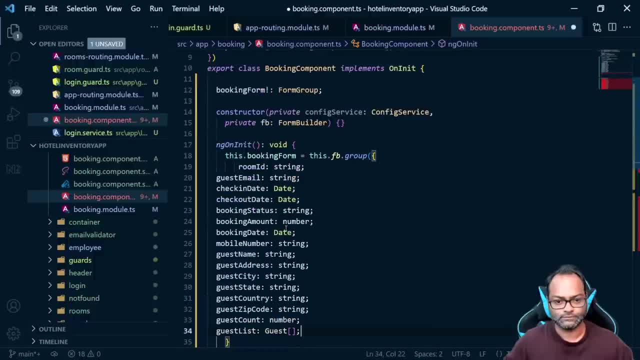 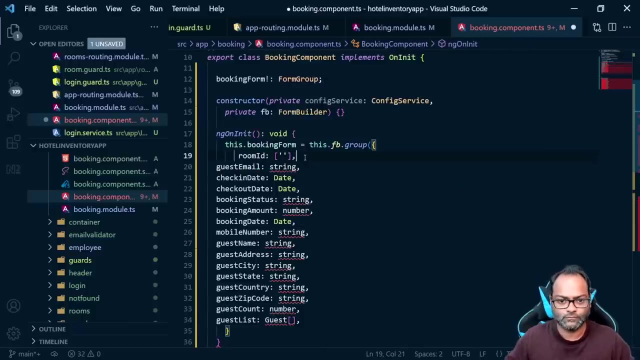 copy andнак this sort, so let's return it to endlessly. so it's a d and unit name and title letter and аХ statement and button ets and date and time setting date وا at the time itself in positive. ok, so let's, Gran, I copy this when: 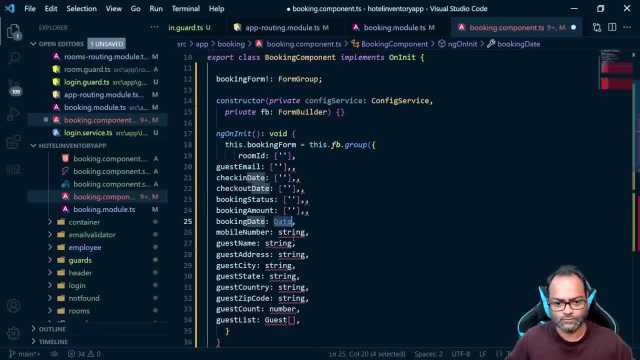 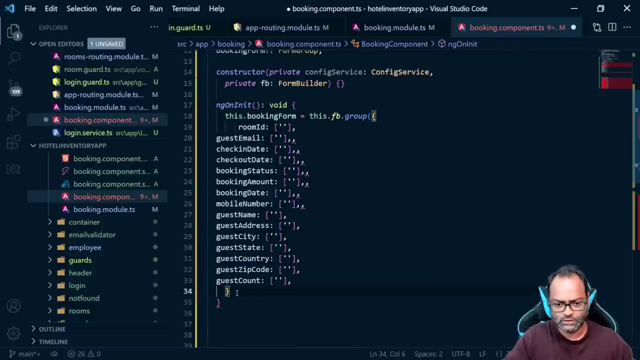 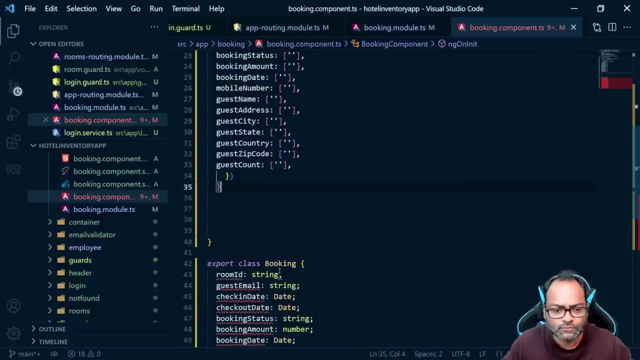 yes, let's give an update and let's see, And we will add this guest list later. So we have this one form group closed here. we'll just remove this two commas with single comma. Okay, Let's format this and somehow this is not close. 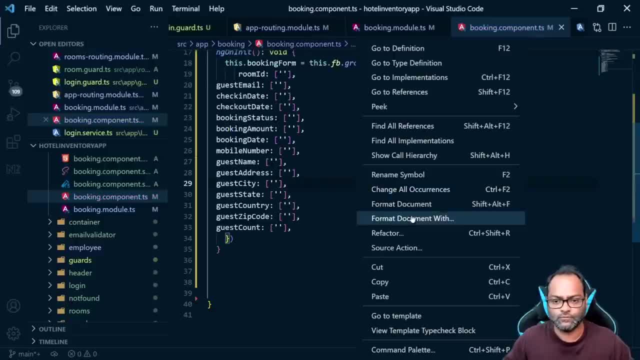 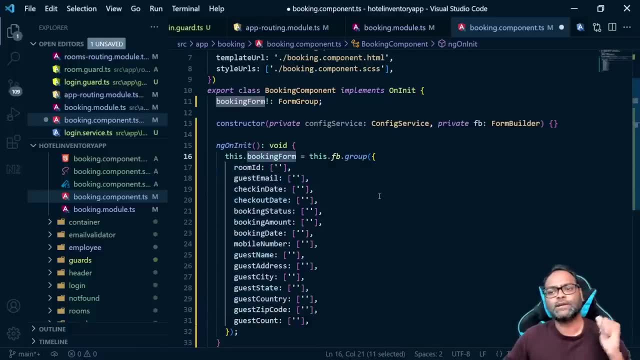 Okay, let's remove this now. So, format document. So we got the form And now we have added some controls. First up, let's go ahead and verify. if this we are talking about, we are saying that this is a form, but is it really a form? 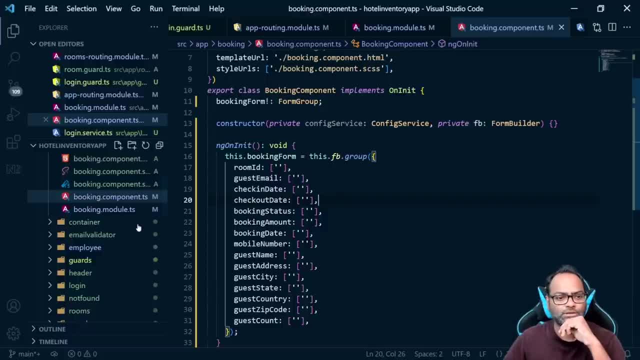 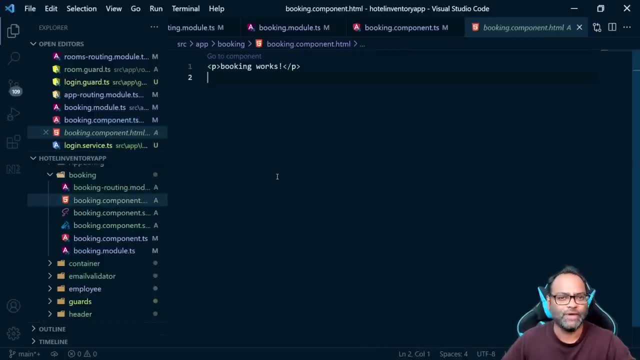 Let's go ahead and talk, see that How we can verify if it is a form. The simplest way is to go ahead and check the properties which are available generally on forms. So remember pristine the d values. So let's try this one. 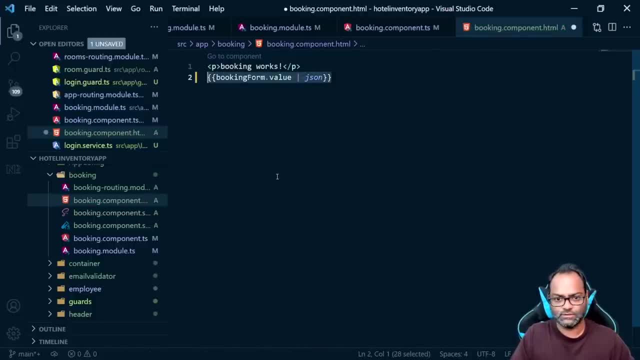 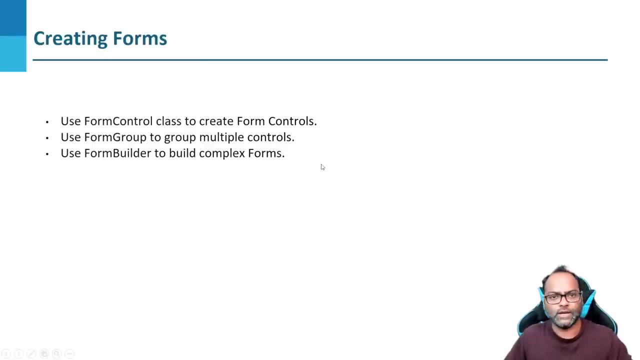 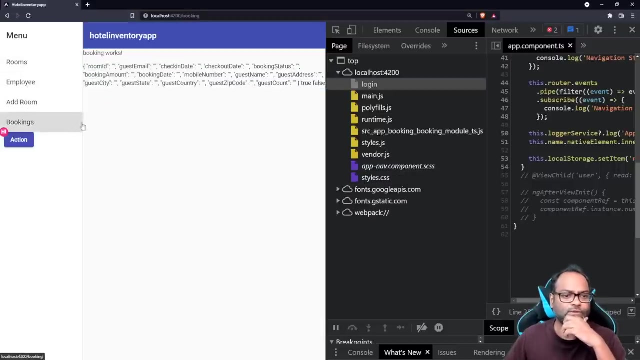 So booking form: dot value by JSON, And then we'll also talk about pristine, Pristine and dirty. Now let's go back to the UI And of course this. this route is not supposed to work, but bookings will And you can see in values. we are getting all the values or all the properties which 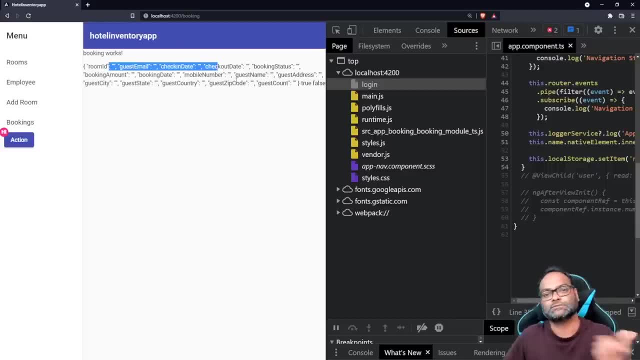 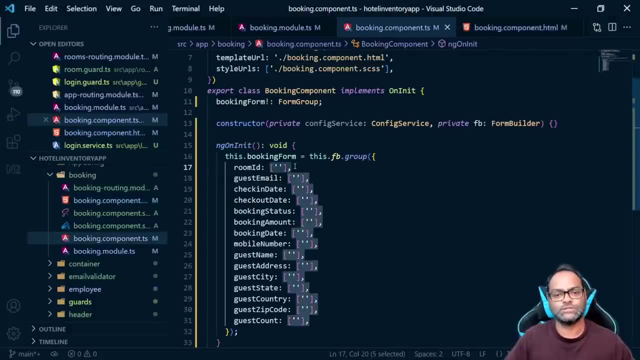 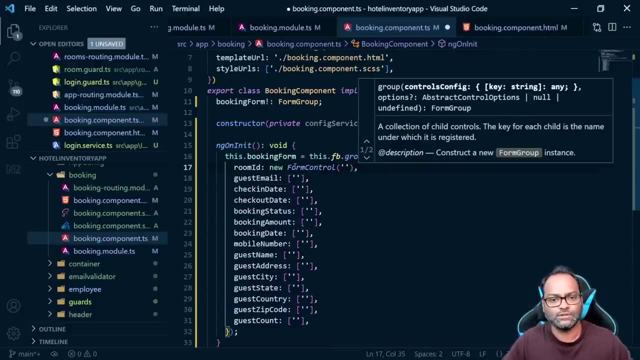 we have defined And all the values are, by default, empty, Empty string. Okay, So let's talk about this first. So this is a shortcut to this one, So you can actually use new form control and provide a default value. So either use this syntax or this syntax. 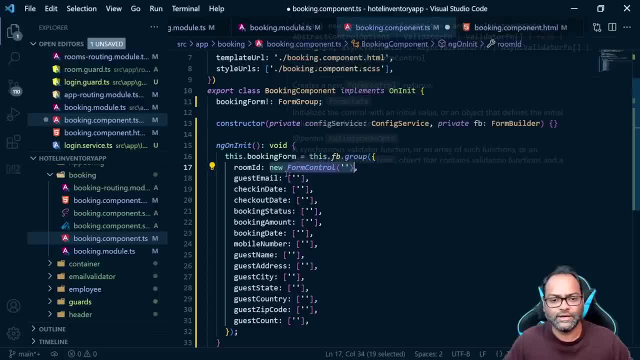 I generally use this syntax because it it is. I mean I I love to tell them: okay, this is a form control and because of typing right, So otherwise you can use a word and use this particular syntax as well. 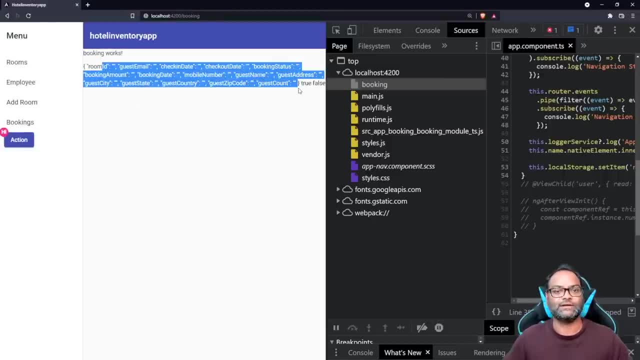 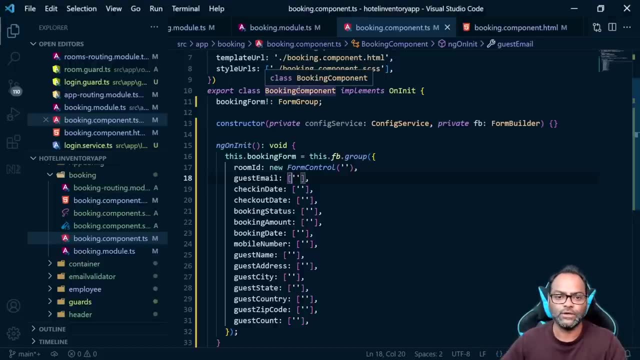 So now we have all the controls defined. So what we did so far is we created a. we sorry, we added the reactive forms model. We created the form using reactive way, by using form group form builder. Now, next thing- sorry, the next thing which we have to do is now we have to go ahead and 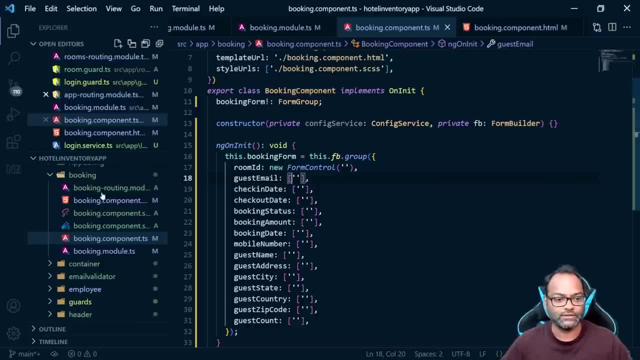 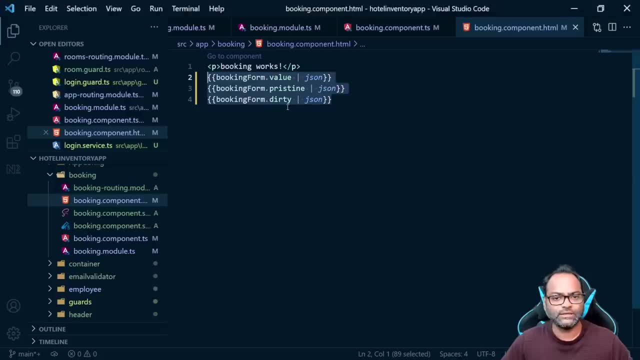 render this form. Remember, as I said, the form is already created and this is the proof right. So form dot value. It means that the form is already created. It means the form is created pristine dirty. it gives it gives us the values as well. 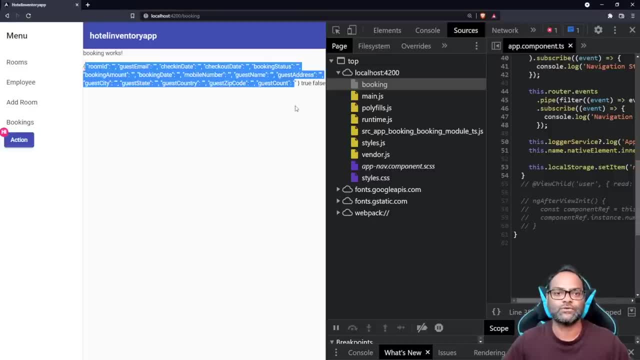 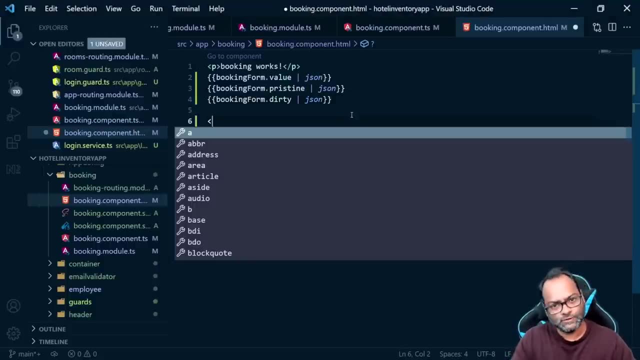 So it means the form is ready. Now the next thing which we have to do is just go ahead and render it. Let's go ahead and bind this form to our HTML right. So how to create a form? Of course, we have to use form tag. 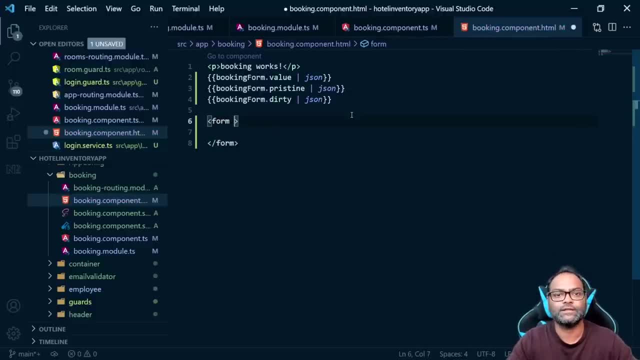 There is no other option. The next thing is you have to define that. okay, now this form is already created, So we have to somehow tell the HTML that, okay, you don't have to create a new form. If you don't, I mean, it will create a new form, right? 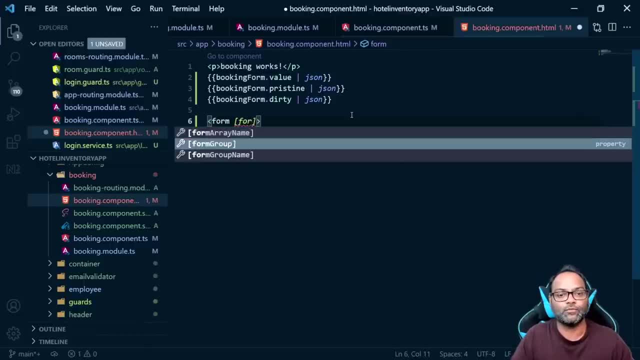 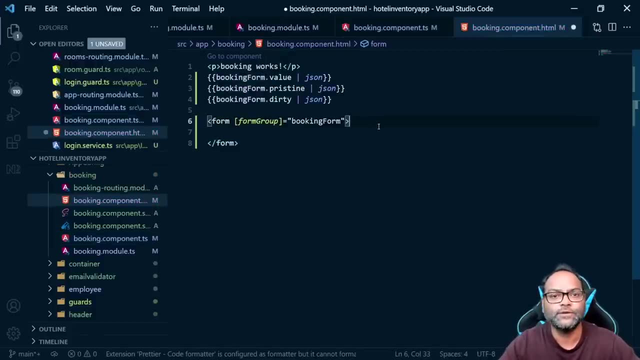 So the way to do is you have to use a directive called form group, And now this form group directive is the booking form, which we have already created. So this line of code will tell the angle compiler. okay, look, sorry, look, we have already created. 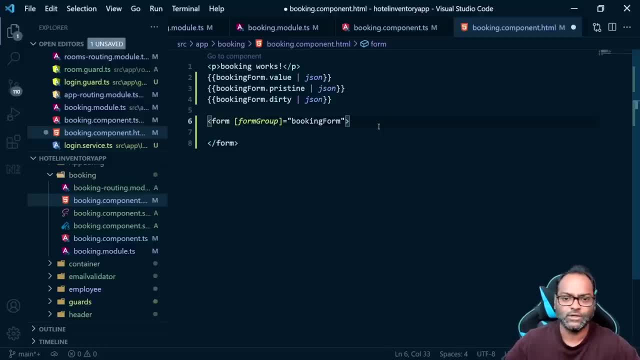 this form. Just go ahead and bind these form to this booking form, which is already created and which has this controls. So step one done. We said that I mean, now let's go ahead and apply a div, but here we will be doing something. 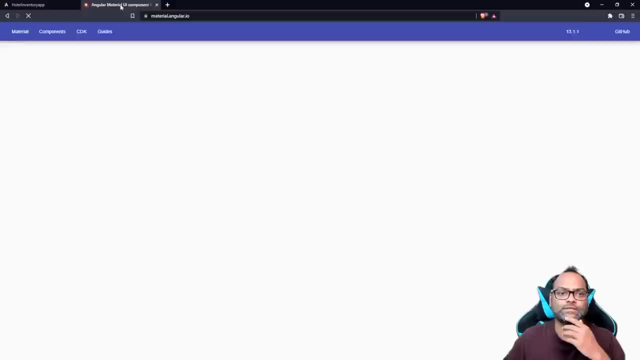 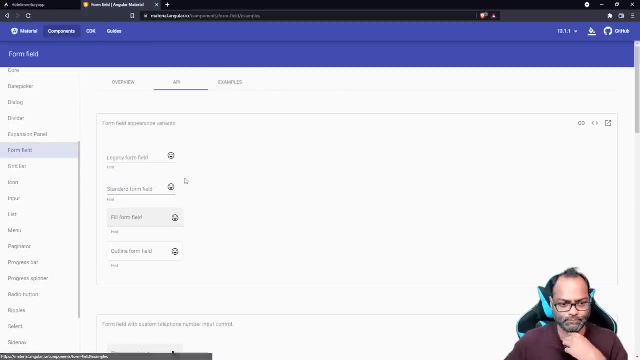 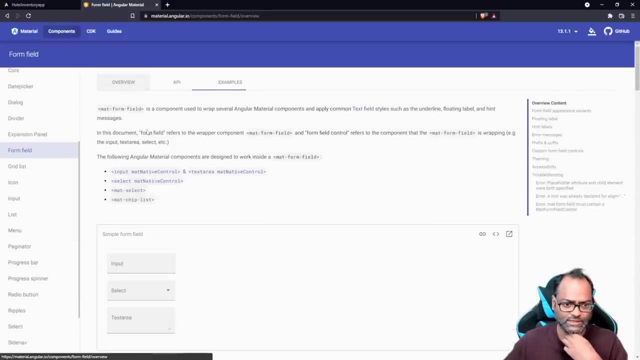 So here we will be doing a different thing. We will be using materials control So we can go to go off sorry components and we can go to form right. So there are multiple ways to add your form input text. So let's go ahead and see how. what needs to be done. 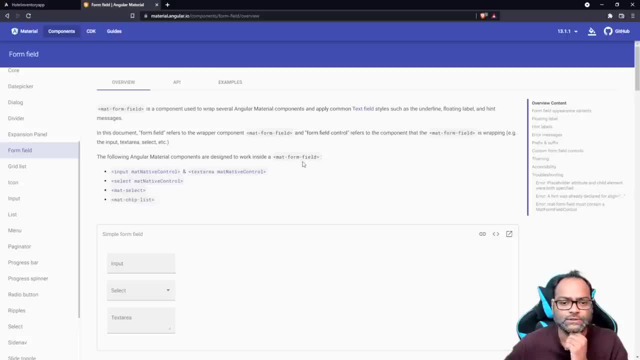 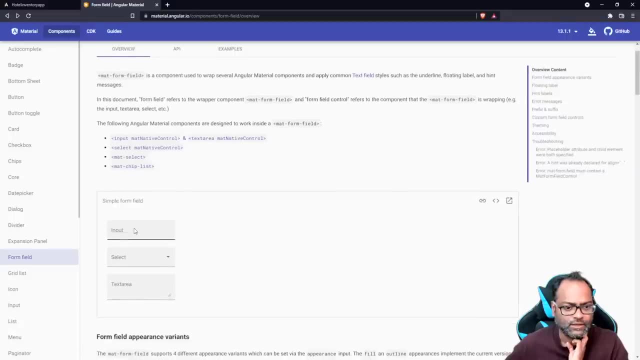 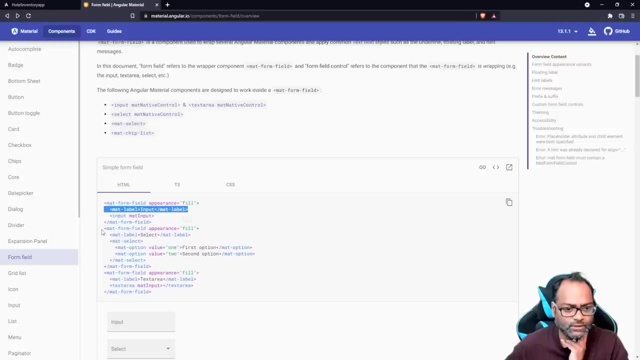 So here, the following element is designed to work inside a module: Okay, So we have a mat form field, So we have- uh sorry- input, We have text area and let's see the code here. So we have mat form field, mat label, uh, select button. 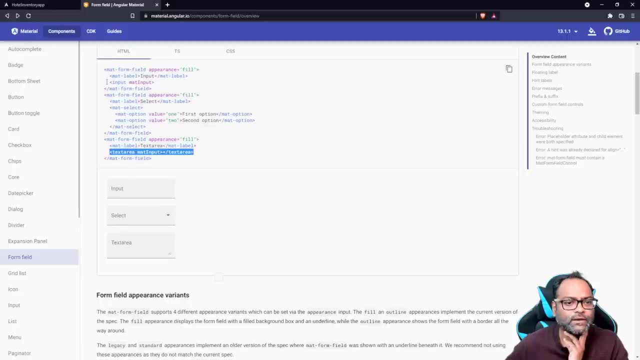 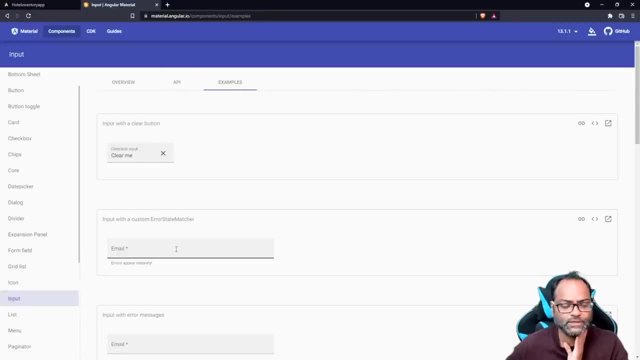 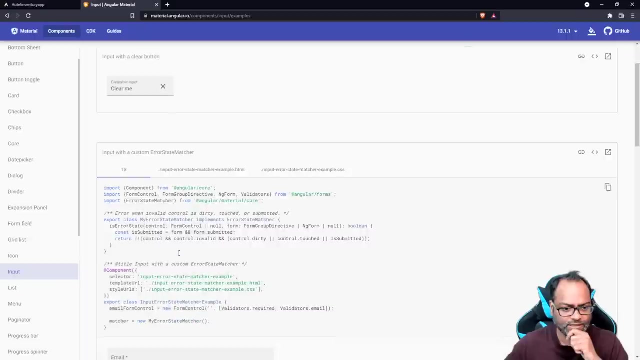 We have text area and then there is should be an input input as well. So we use mat input here. So for input we'll be referring this, but this uh mat input can be wrapped inside the form field. So we have to actually combine both the APIs and we can see it here: uh, HTML, right? 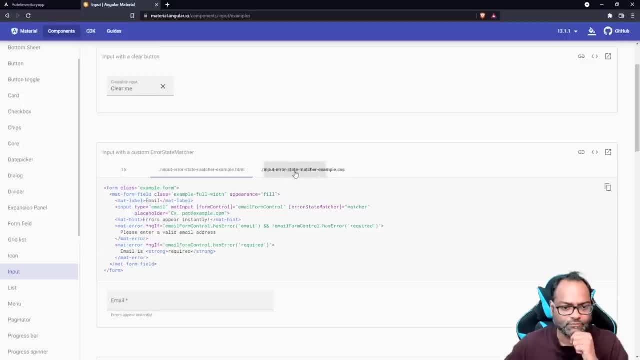 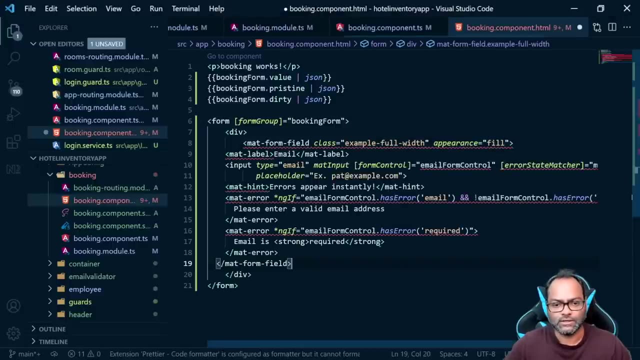 So we have this mat form field class and we will copy the CSS as well from here. So let's do that. I will just copy one and then we will repeat it for this. So here, uh, now we are getting some error. 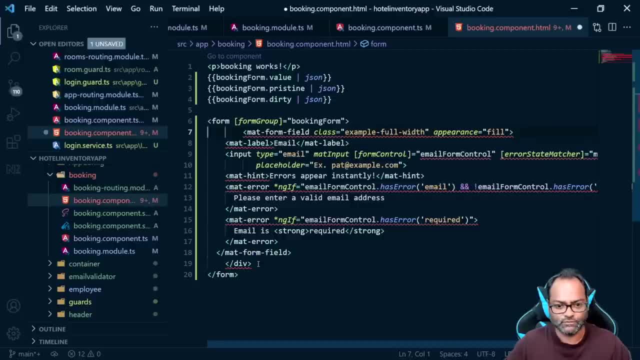 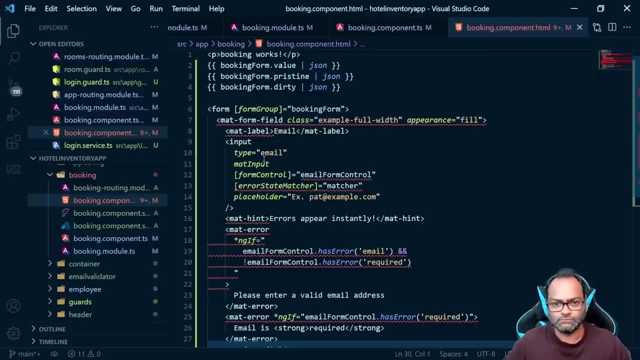 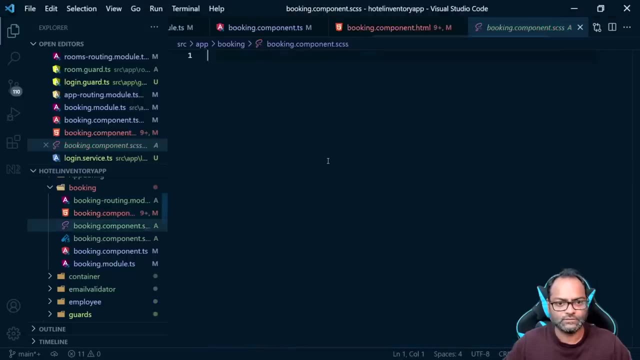 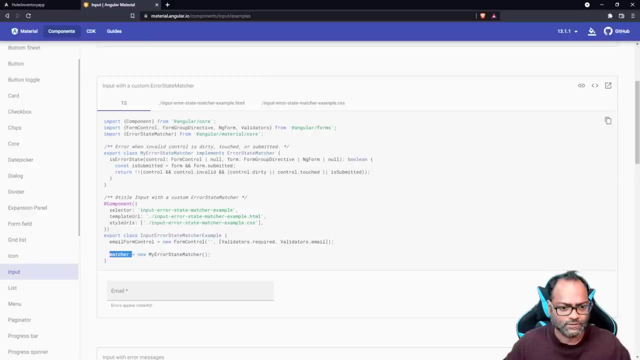 We'll just remove this. Let's get rid of this div now because, uh, here mat form field is what we are looking at. So I'll just say for the document and just ignore about the other. we'll fix those. We'll copy the CSS from here and so the they have some. my uh error states: 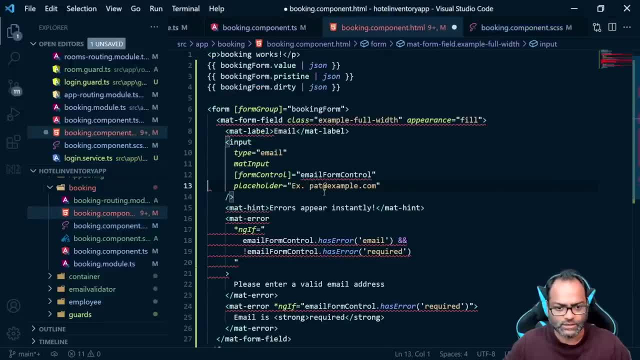 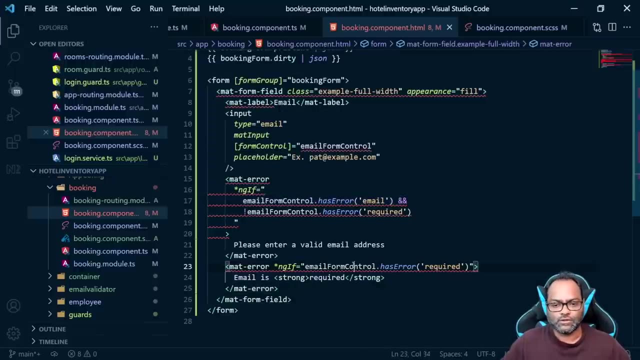 Okay, We'll remove this. We'll not make this much complicated and remove this one from control: is what we need. Mat label: is what we need. Mat error- Okay, I'll remove mat hint- Mat error- Okay. And now let's talk about this. 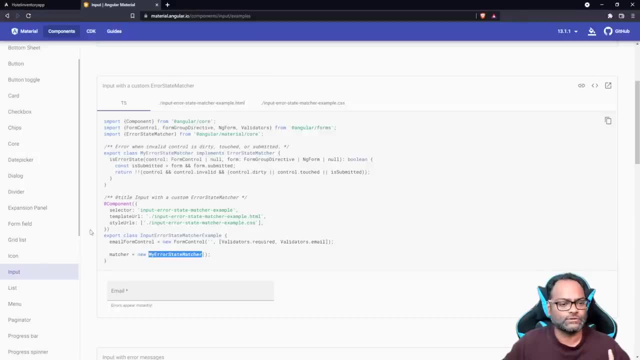 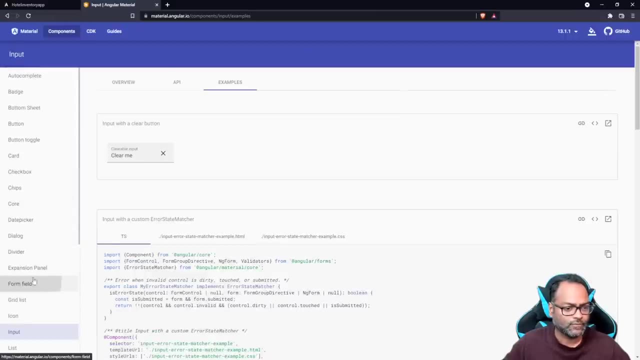 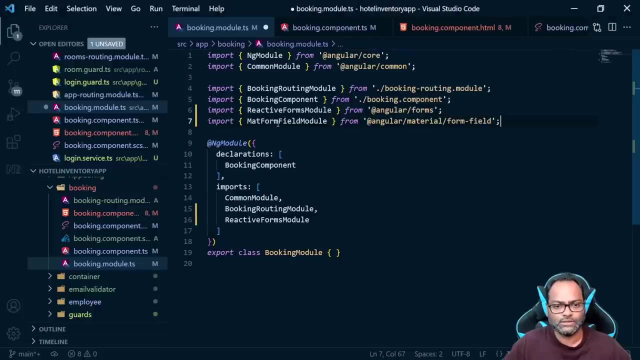 So here, uh, what are the APIs which we are going to use is mat input and mat form. So let's go to the form control, form field control, and let's see what we need to do. So we need to import this mat form, mat form field module. 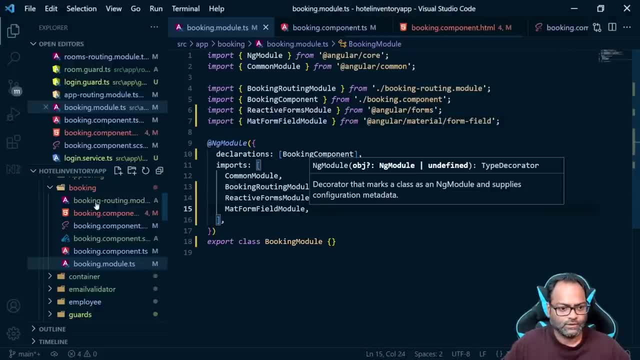 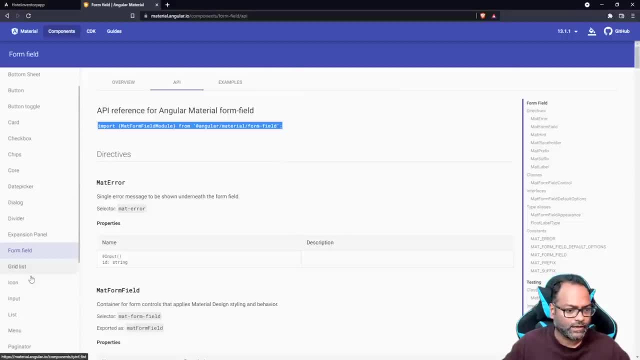 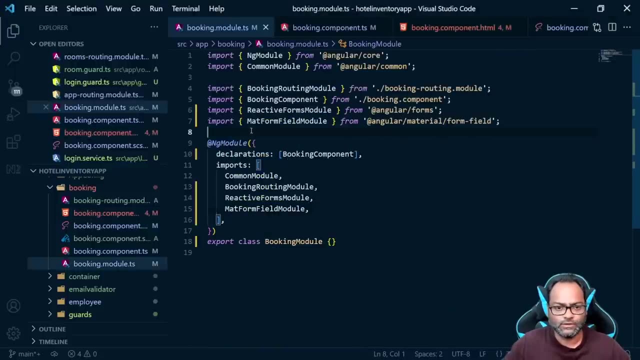 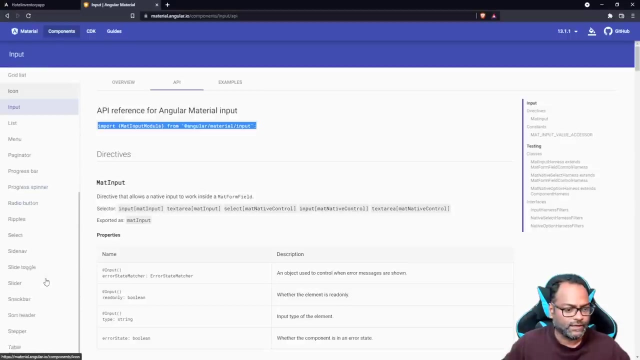 Let's go ahead and add it. Okay, So now mat form field error should be gone. Then we have label and input. So let's take input second, and now all the errors related to input should be gone, And then we had label. 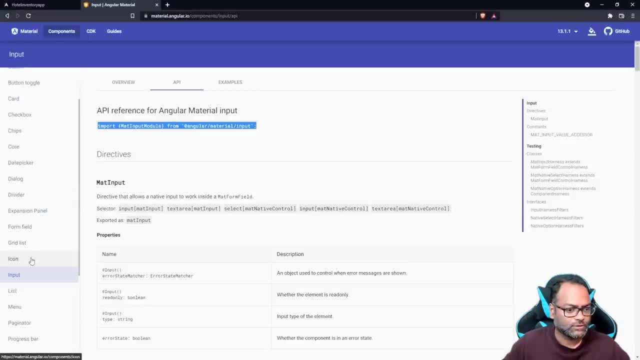 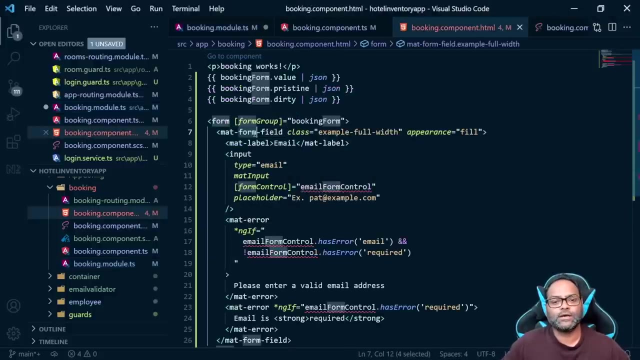 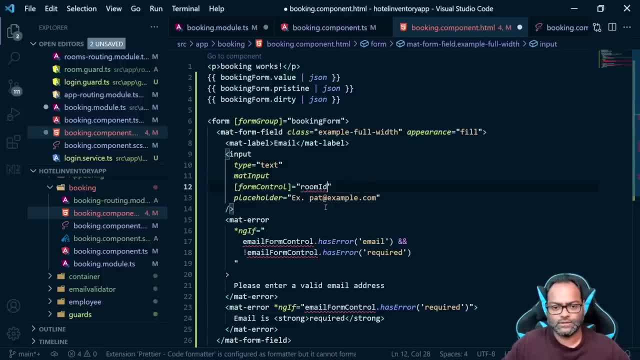 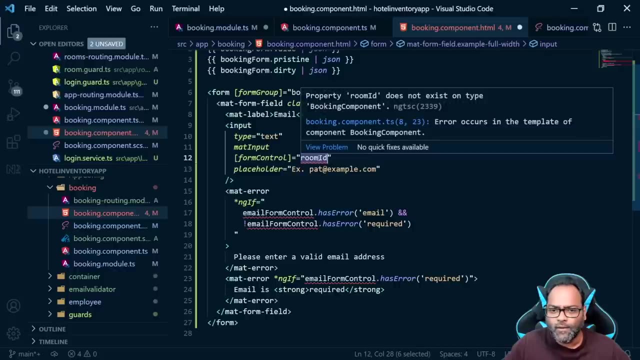 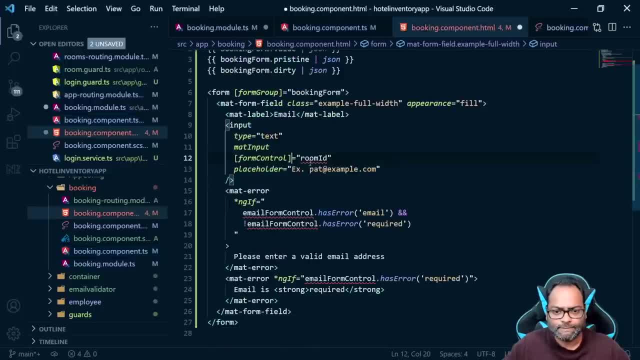 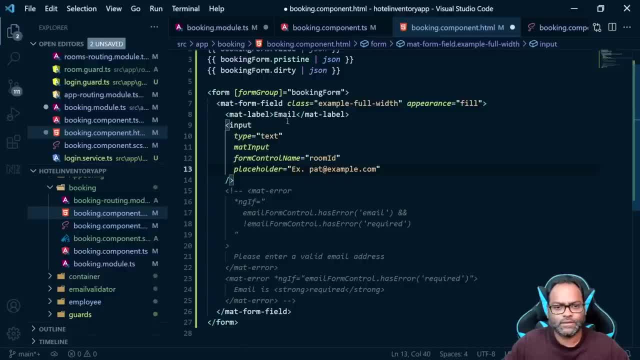 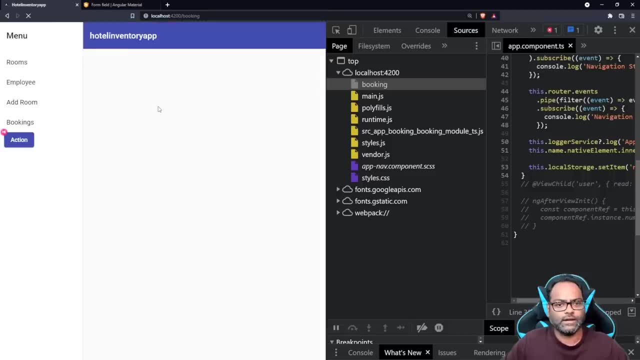 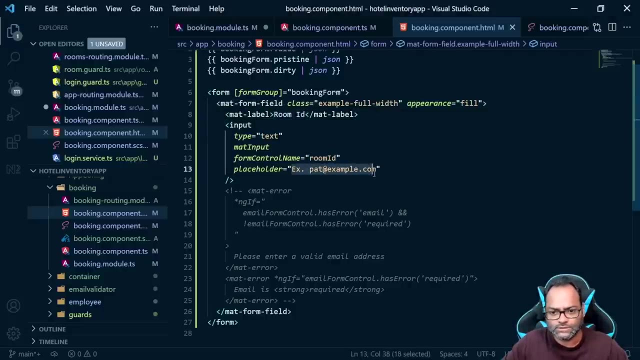 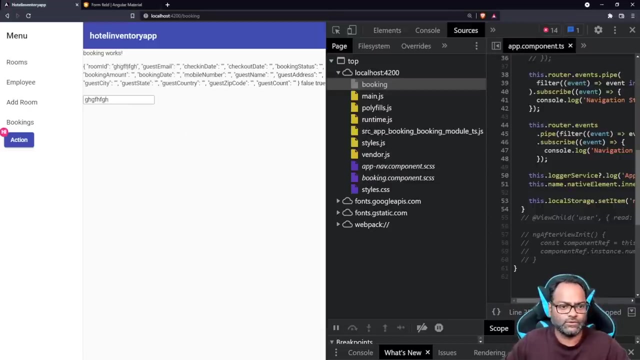 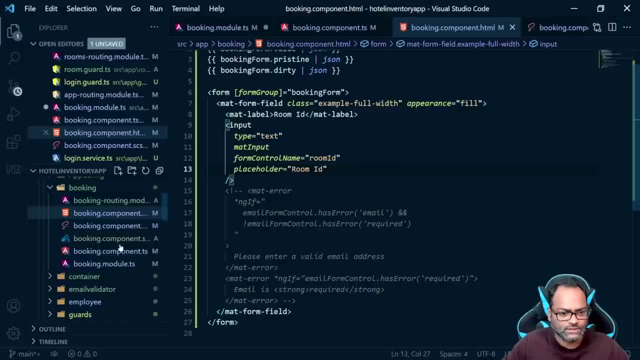 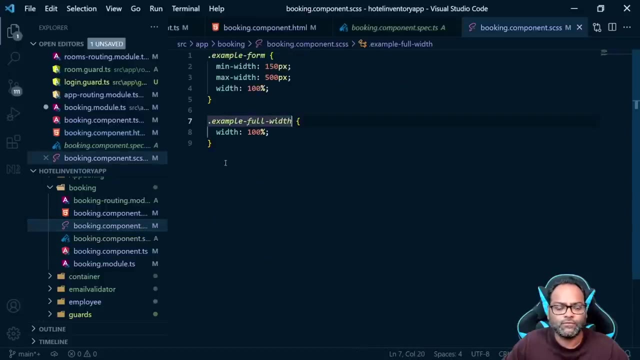 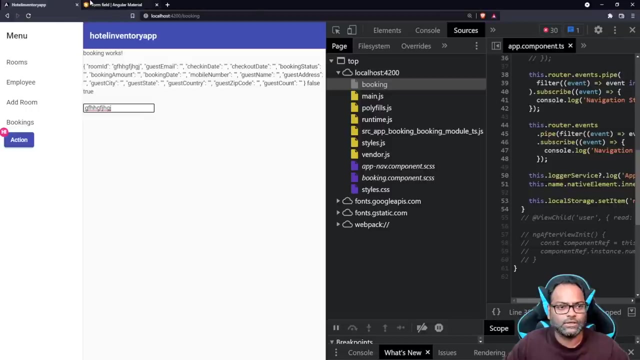 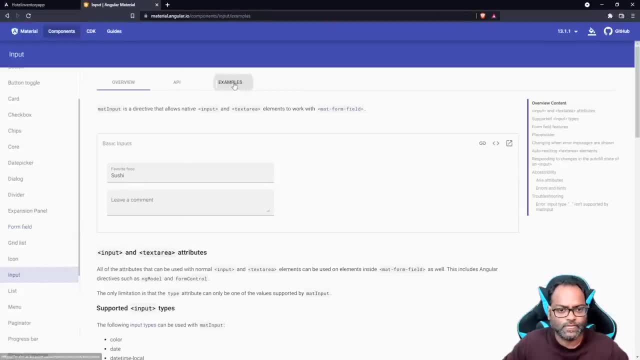 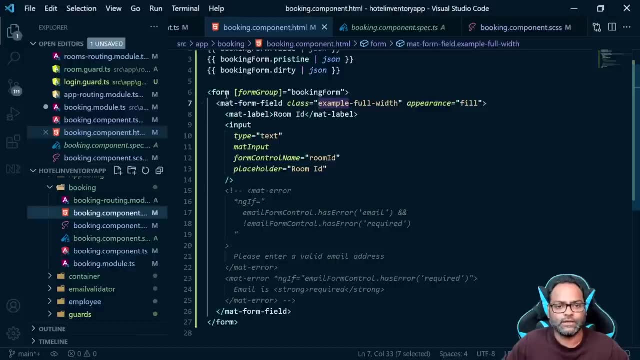 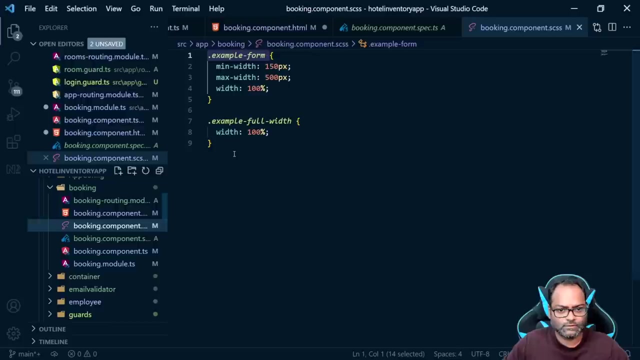 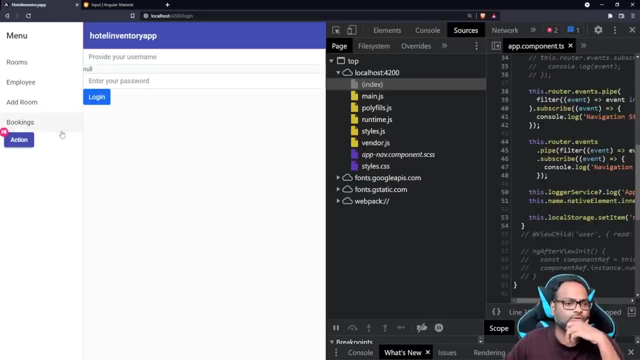 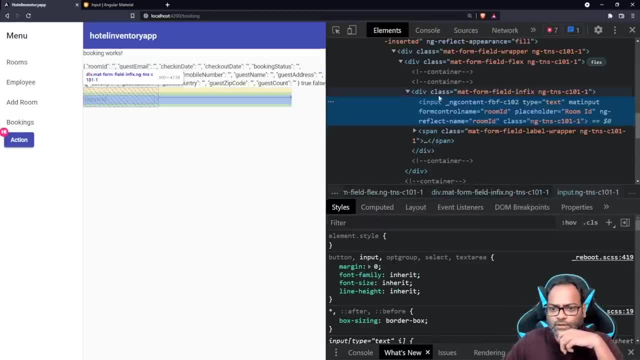 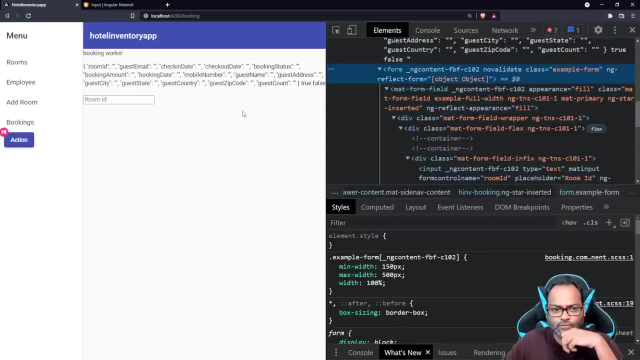 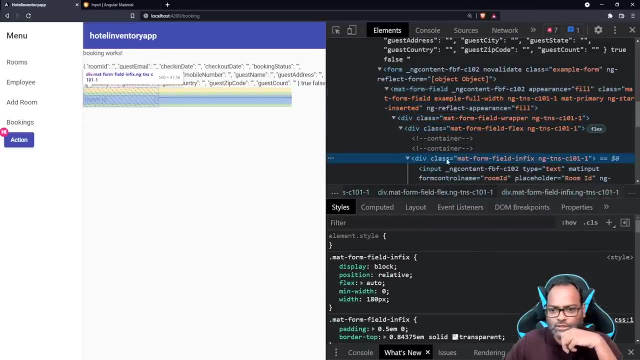 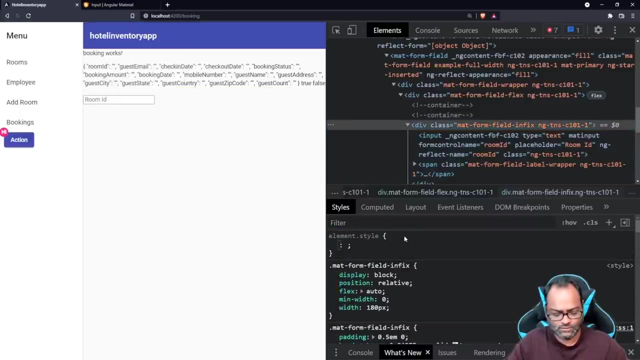 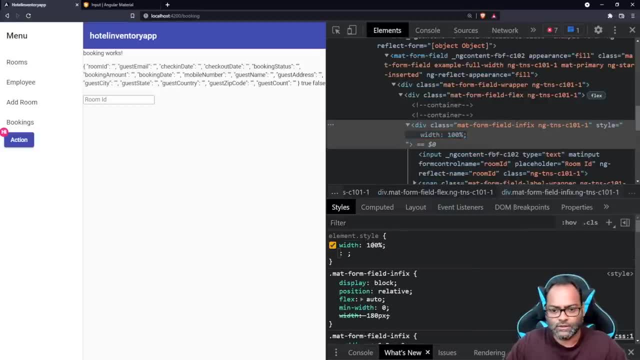 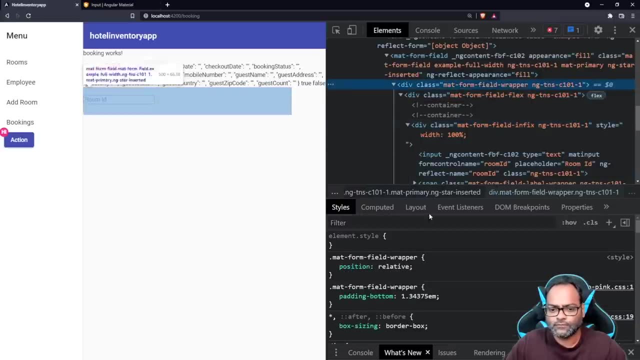 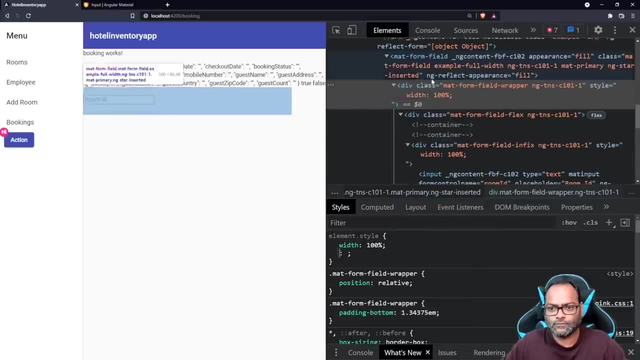 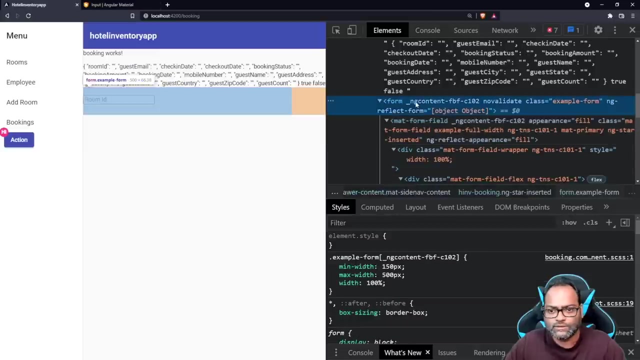 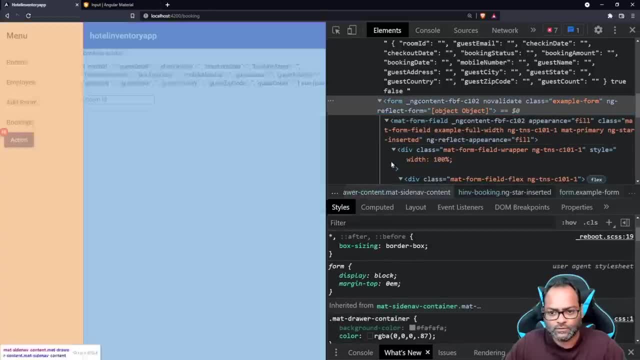 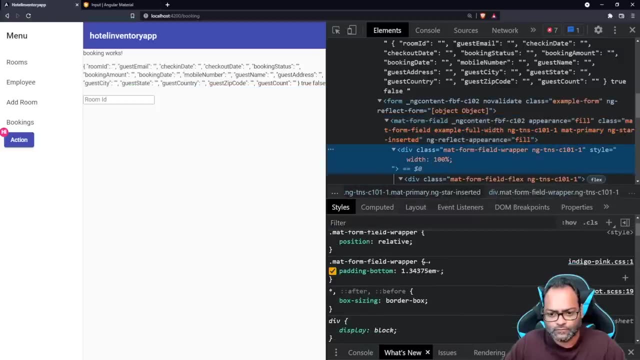 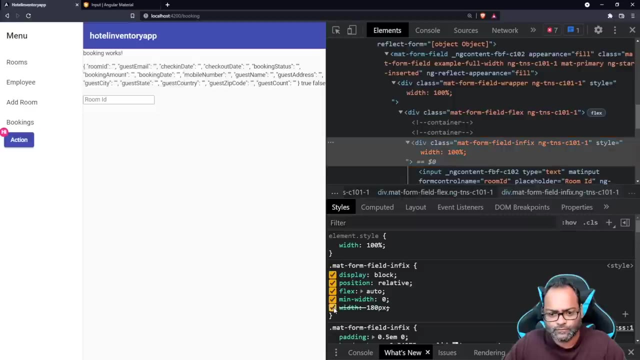 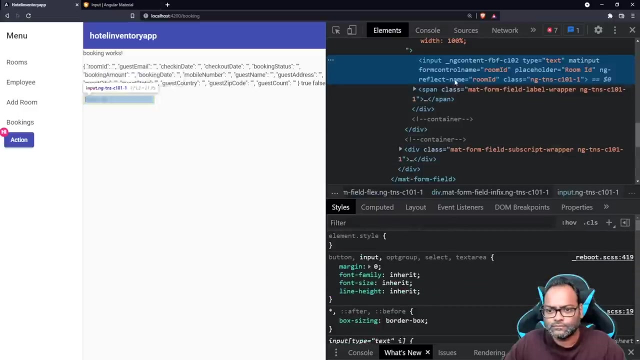 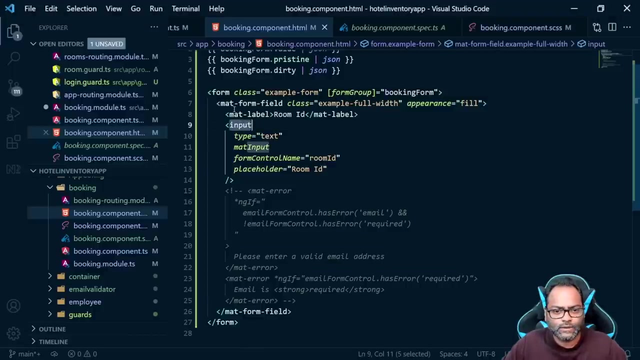 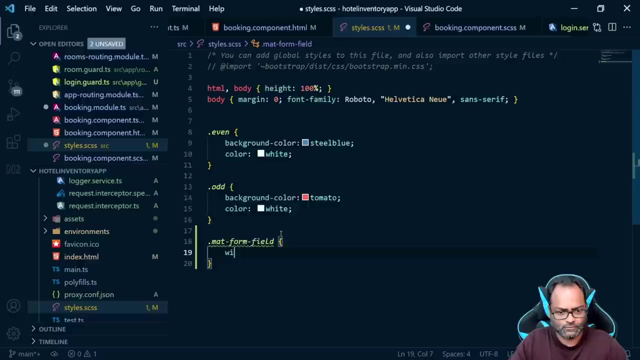 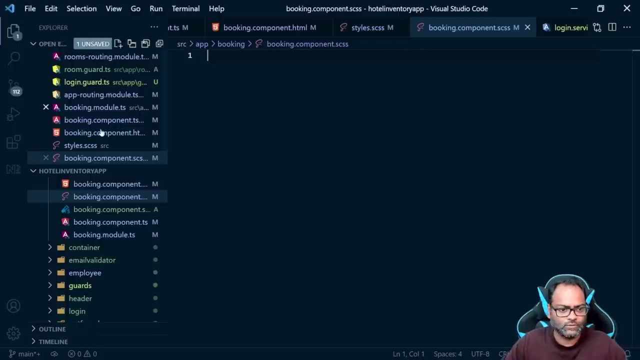 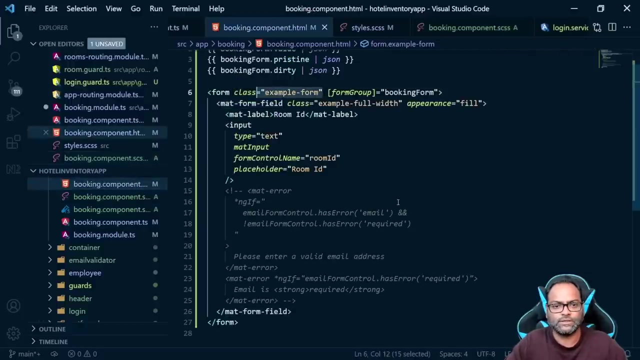 Okay, Okay, Okay, Okay, Okay. Thank you, Let's try to do this. Let's add it in global CSS. Okay, still not what we wanted it to be. So let's remove this And let's remove, Let's remove this- classes as well. 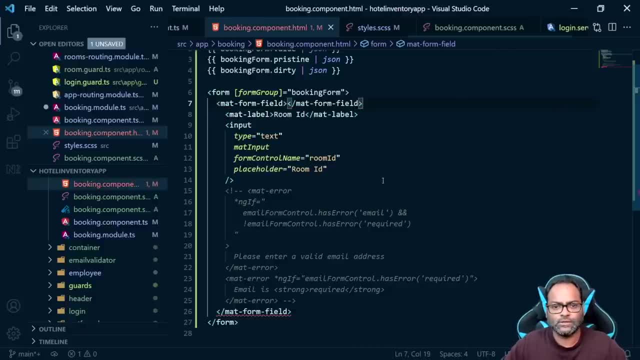 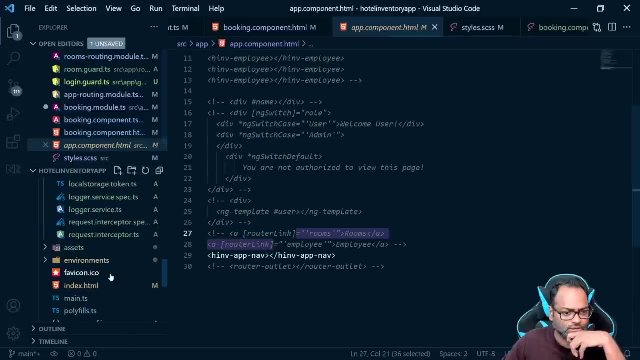 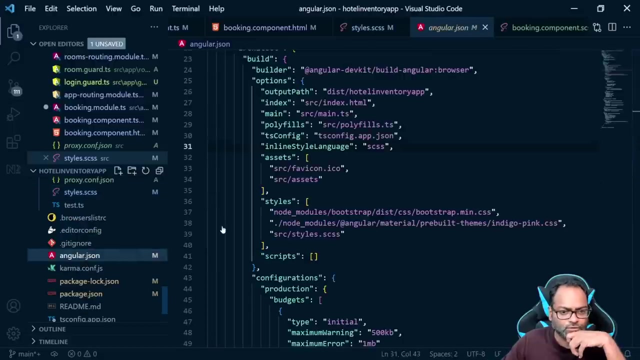 And let's remove this appearance as well. Okay, So we have this form field. Okay, somehow it is not even applying the material CSS. So let's go ahead and see. So we have the styles available here, And And let's go to angularjson. 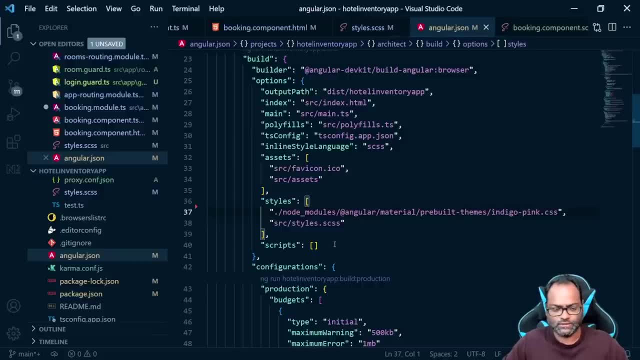 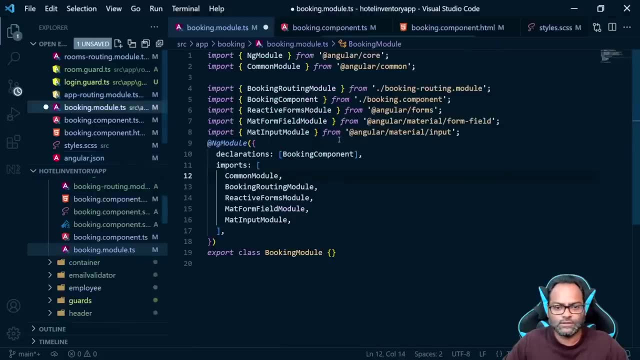 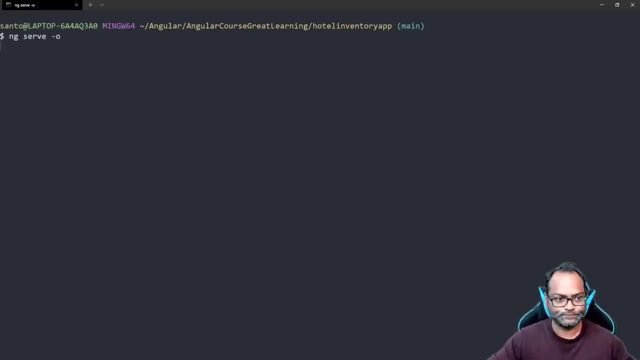 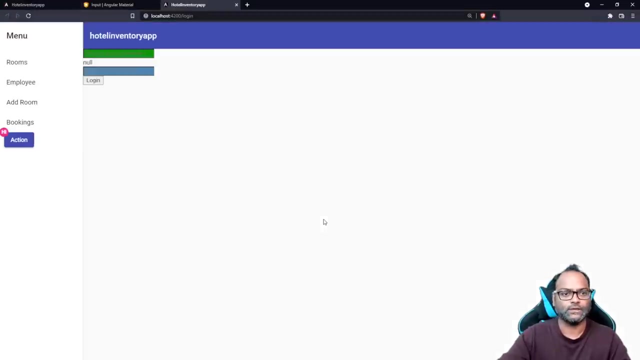 Indigo pink. I'll just remove this bootstrap one for time being And let's restart the server. Probably, as we are using both, it is actually causing a conflict, So let's save this. Okay, let's see if it works now. 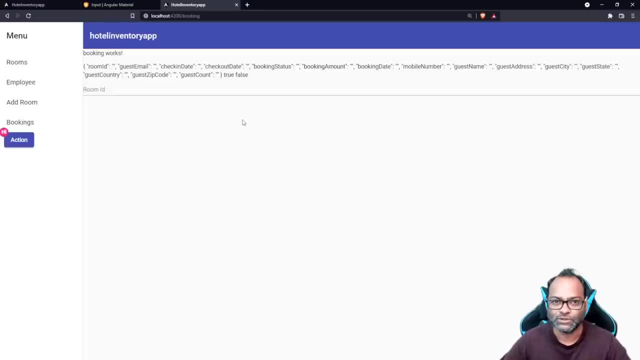 Okay, so I was right. So it was just due to the conflict, because we are using both Angular Material as well as Bootstrap CSS, So now you can see it has room ID And this is how you are actually material component. Sorry, Sorry. 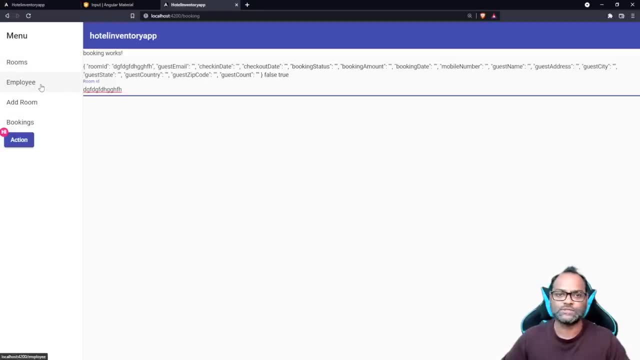 Material control should look like. I'm sure other forms is broken now because we were using Bootstrap, But we can. We can actually replace everything with material control. We'll do that. We'll do it. I mean, you can try it as a practice for other controls. 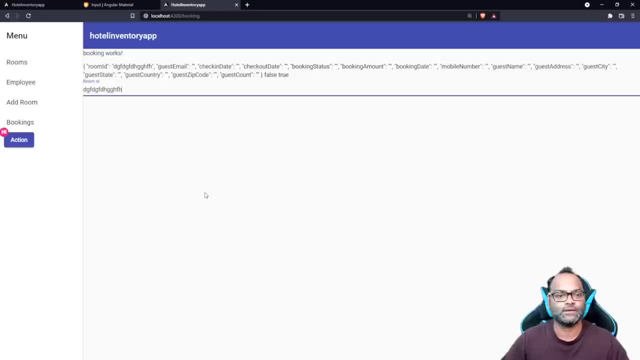 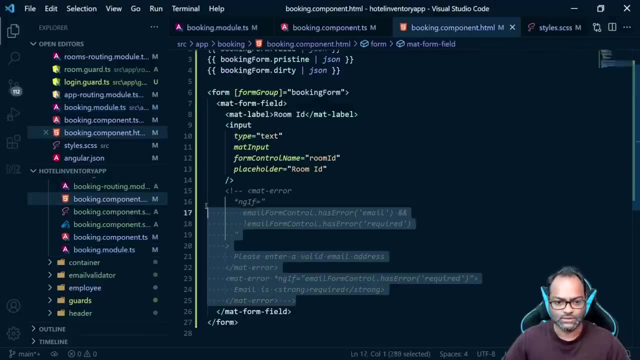 But here we'll be using just the, Just the material form. So let's go ahead and add other controls. So I'll just remove, I'll just keep this, But I'll just go. Okay, Let's do it for mat form field. 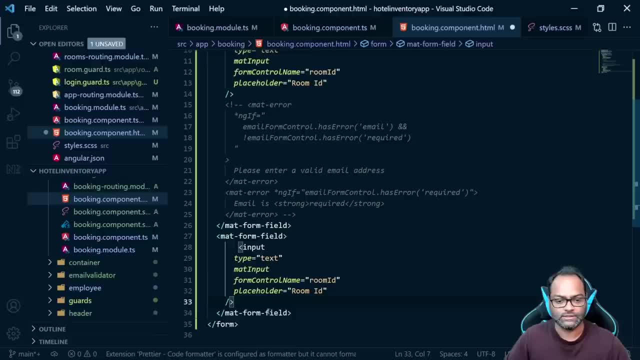 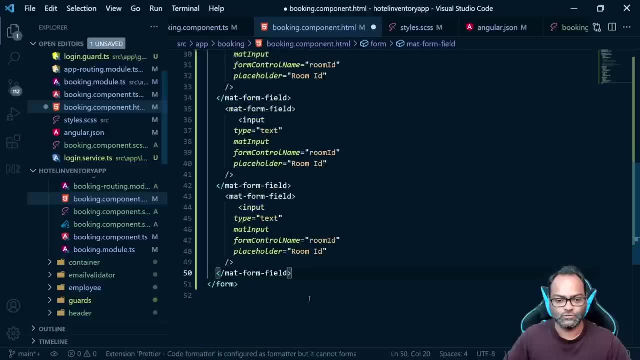 And then we need an input control, Right? So we'll just add this and then we'll replay it, Just so. we have a lot of controls. So let's do a copy paste as of now, And then we'll see which control to use. 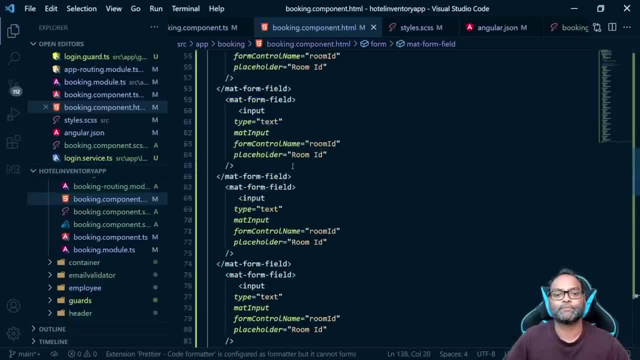 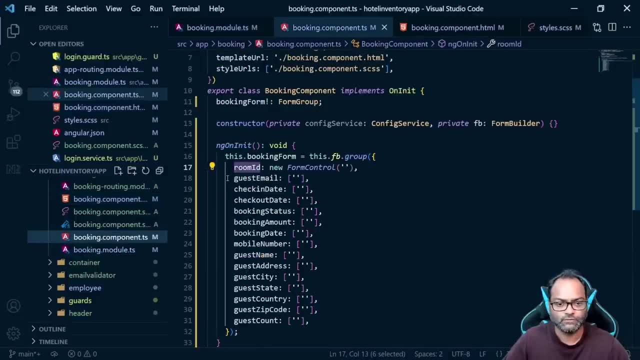 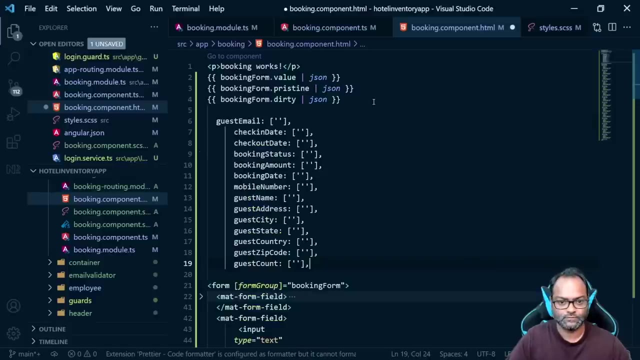 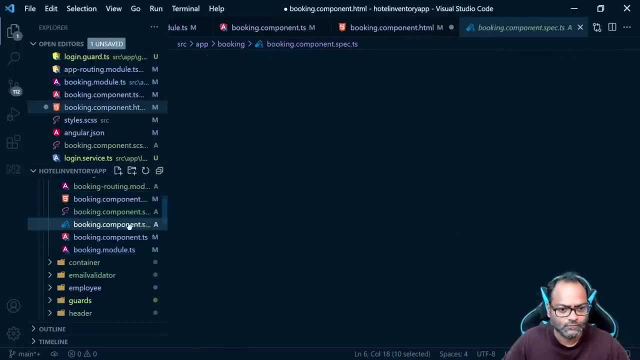 Right, We'll just need to figure that out. So we The first one, Let's open the model. So we have these many controls And let's put it here. So I think not everything was copied. Let's see, Okay. 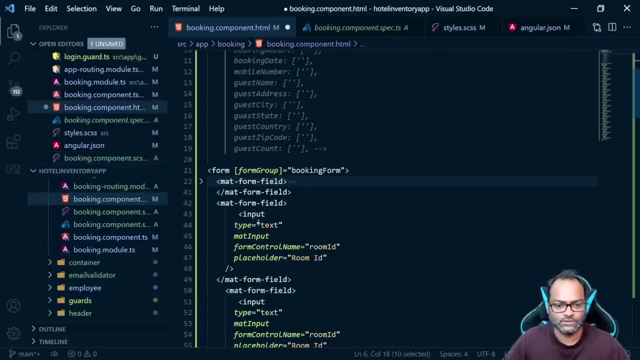 Room after room ID. So we need to guest email. So the next one is: type is email. Okay, So Guest email, And we'll say provide And Email. Did we have name? Okay, Sorry, So name should be. 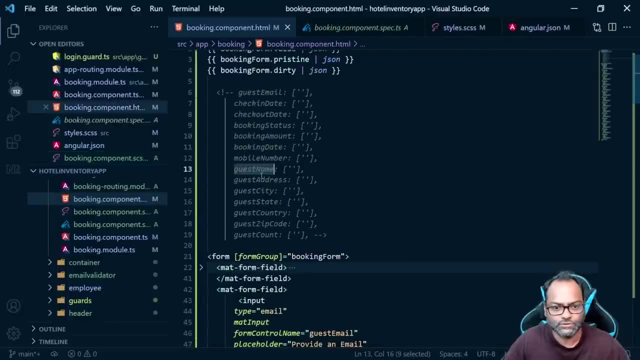 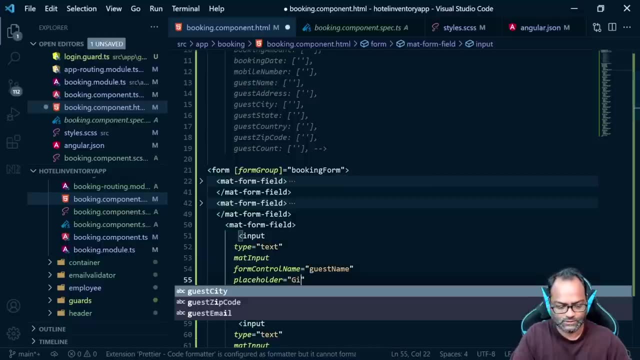 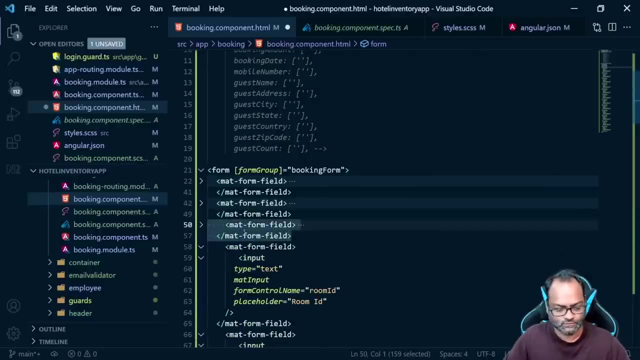 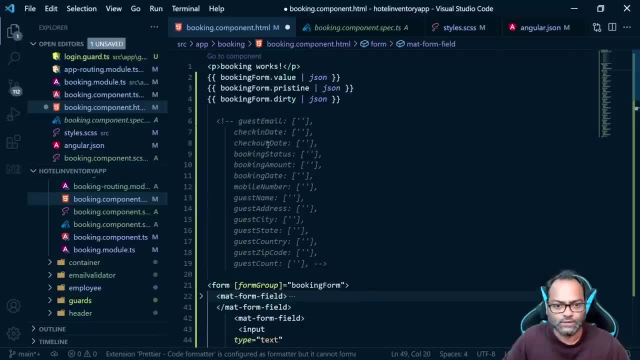 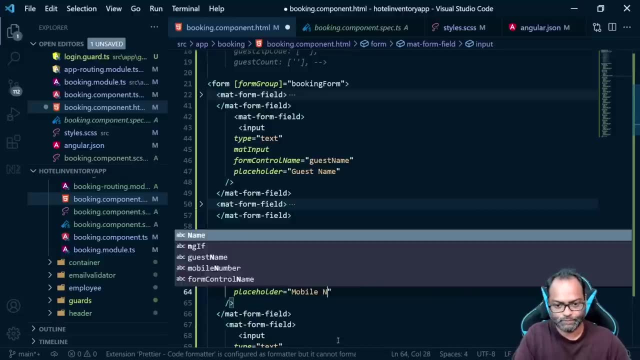 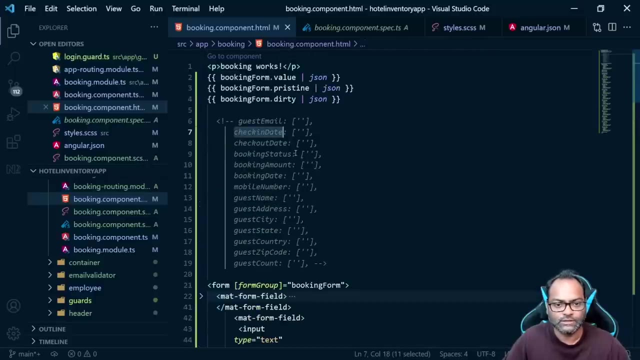 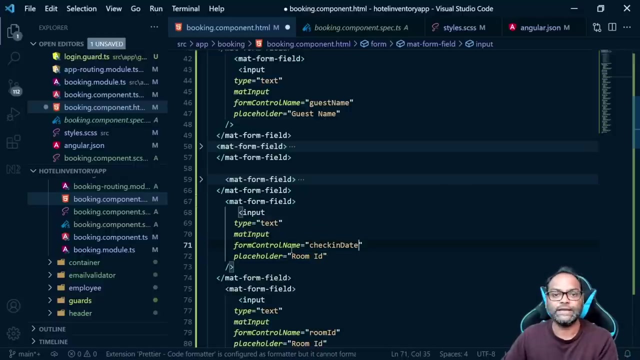 So Now we can have other things: which is mobile number, So this is mobile, And then we have, So we'll check in date, So we'll know if it is this form control, name, checking date, But interesting, So checking it. and second checkout date. 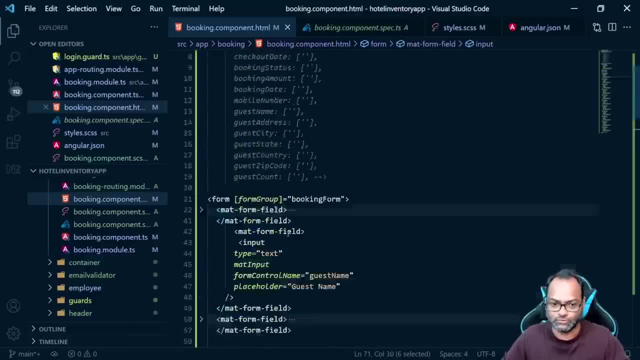 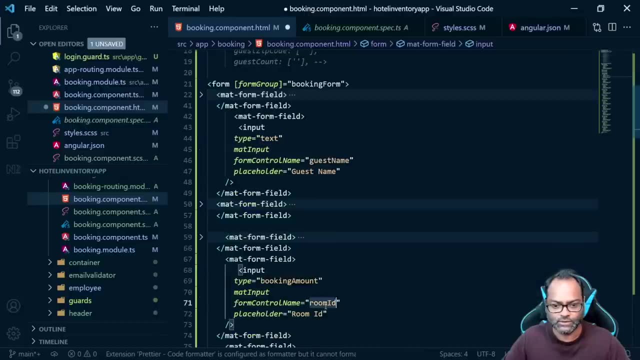 Right, We need control. I mean control, so we'll use date picker booking status. we will see it later. booking amount. booking amount and type is number, because it's an amount. booking amount. booking date: it will be again date picker mobile number. we already did. 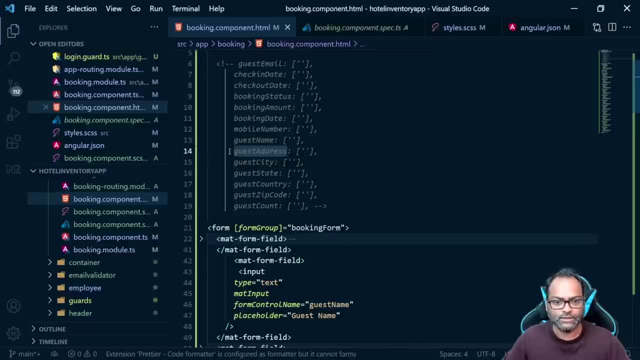 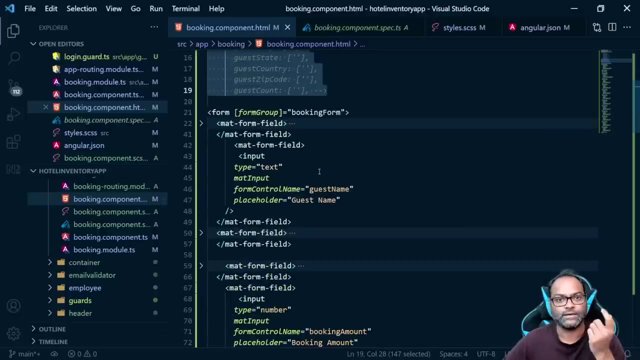 and then we have guest address city. let's do it later because i can see- uh, i think this can be another form as well, so we'll see that i mean we can- how we can actually put this entire thing as a different property, as an address. so let's see that later on. let's wrap it. 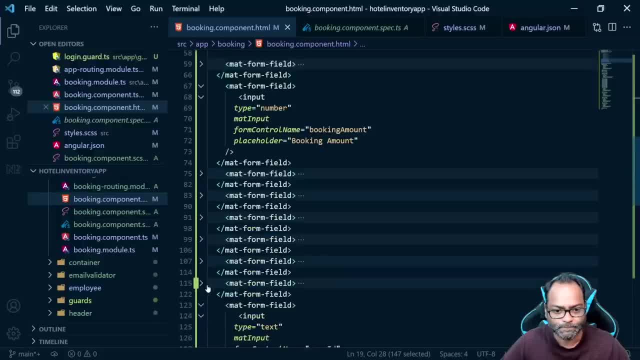 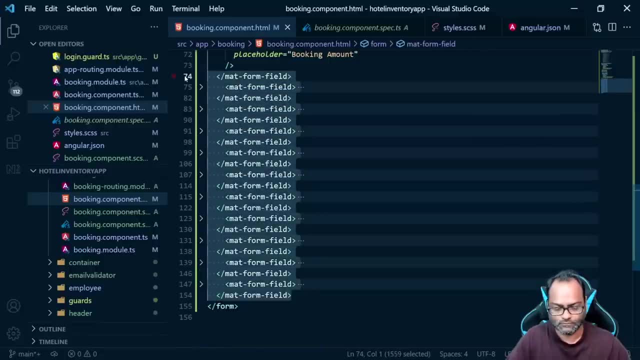 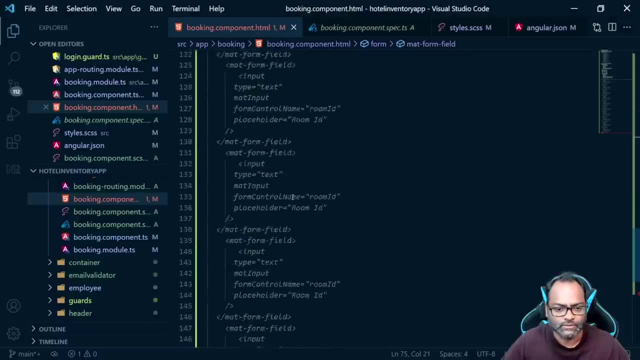 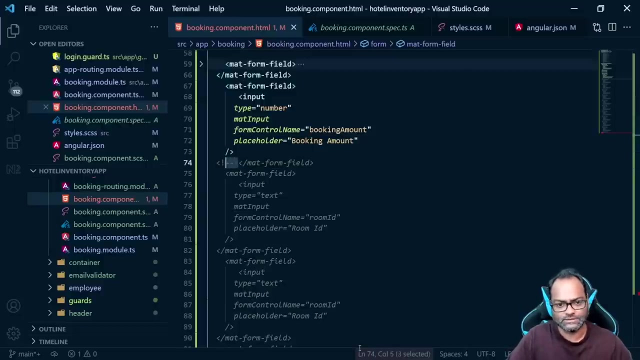 by commenting the other controls. okay, as we are going to need it, so we'll just keep it here and let's see our form. okay, unexpected tag of. looks like i commented the form as well. okay, it's here, but something, something which is not closed properly. yes, here it is okay. so now we have room id, guest name, email, phone number, booking. 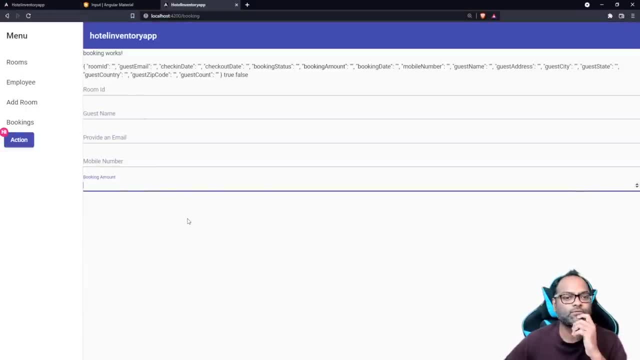 amount. so these are few properties which we have. let's enter so we can see: okay, guest address name. and then we have guest address. now let's see the guest address name is something which is getting updated here. email is getting updated here. my number is getting updated, uh, here. and then we have booking amount, which is also getting updated, just to verify the 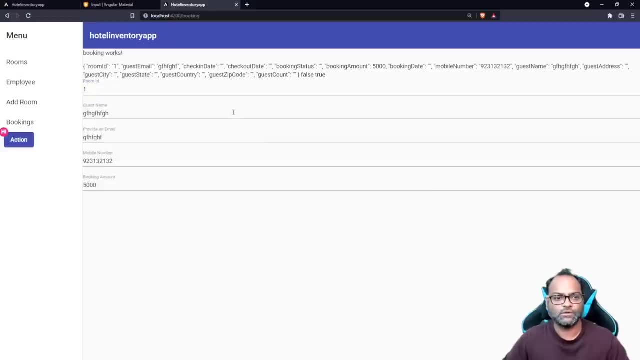 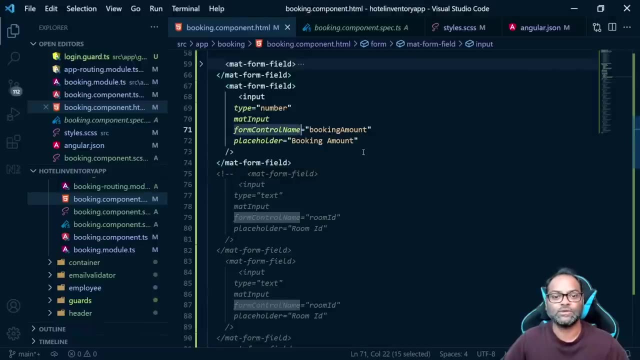 form, i mean if everything is fine or not. so done so all these properties are actually mapped to its respective controls right by using something called form control name, which maps this uh input control to the control which is already defined. next up, we need date pickers. let's take 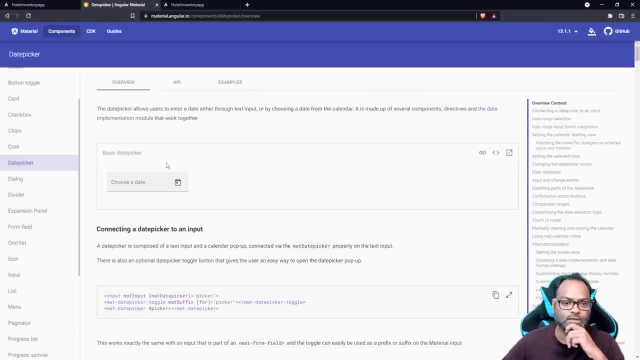 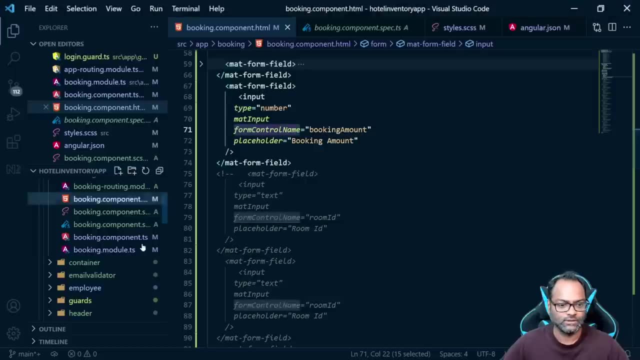 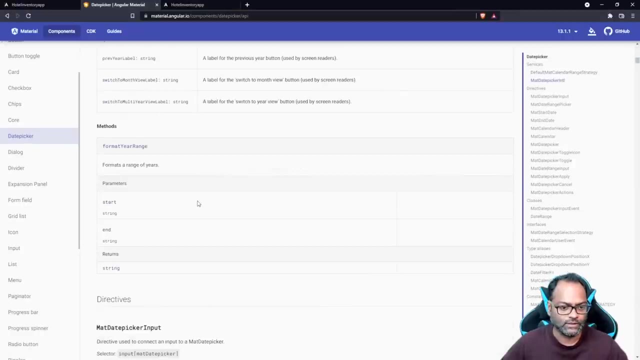 it from here. so we have something called date picker available here and which gives us some nice state picker. so let's go ahead and see the api so it says, okay, you have to add this, you have to add date picker module. so let's do that, and do we need to do anything else? the answer is: 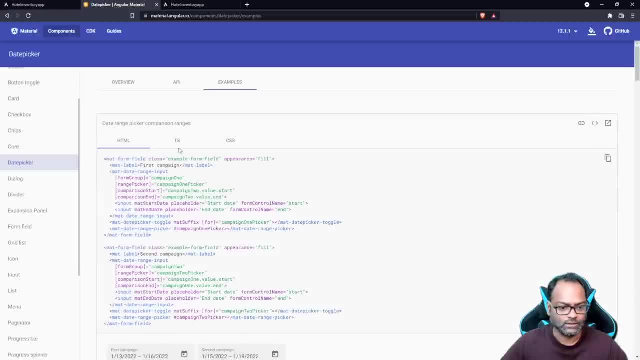 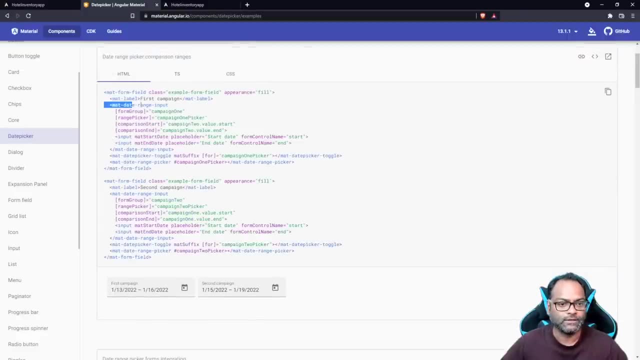 okay, no, no, let's see the uh uh here. um okay, no, so we don't have to do anything. we we can just use mat. there are okay. there are two things. uh, we also have range. do we need range? the answer is yes, we could. we can actually uh provide start date ended by using the. 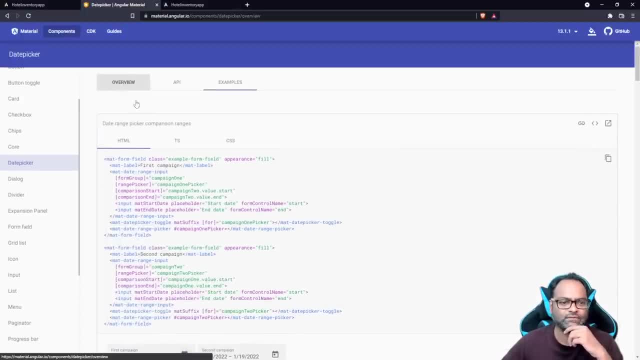 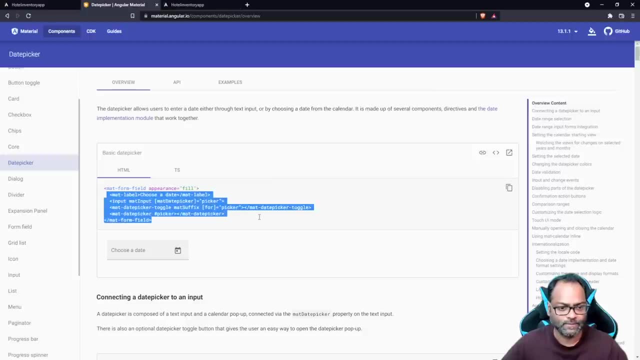 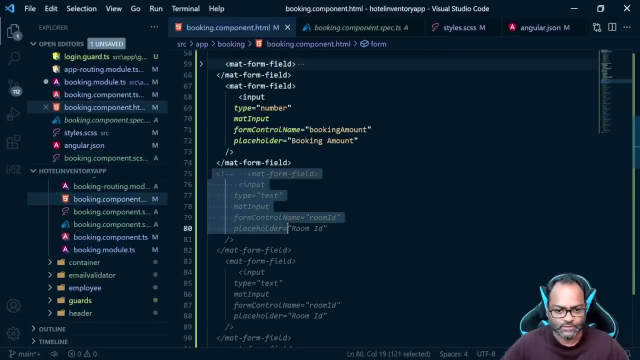 range control. but let's, let's see. we will use the date picker. so we have two different properties. so here mat date picker. so let's see how to use it. we already have this mat form field. i'll just comment the first one mat form field from here to here. okay, 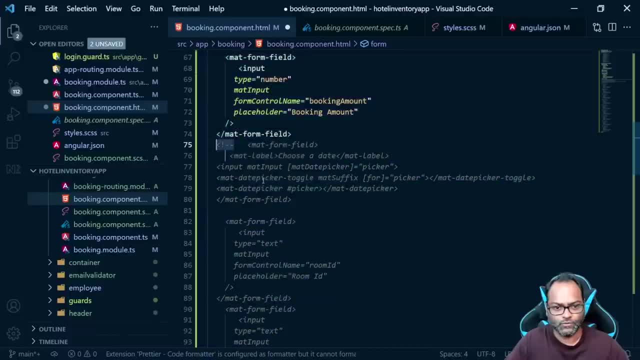 let's copy this and move this commented thing to here. okay, so we have mat date picker, which is speaker. uh, what we need to do is we need to map, the map, the control. so we will be using here form control. name is equals to. we have check-in date. 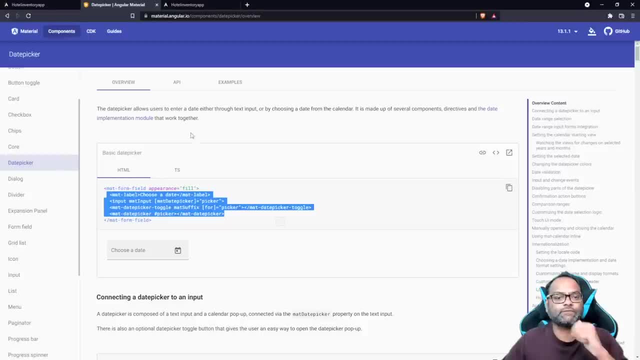 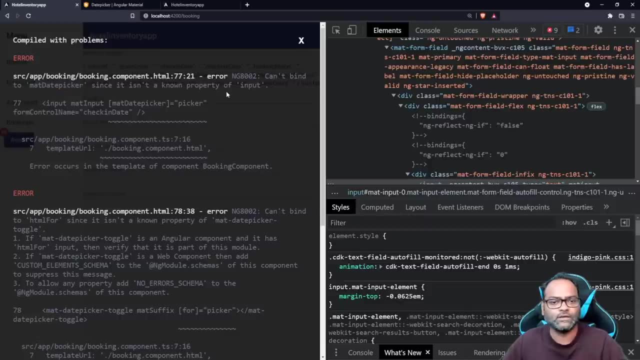 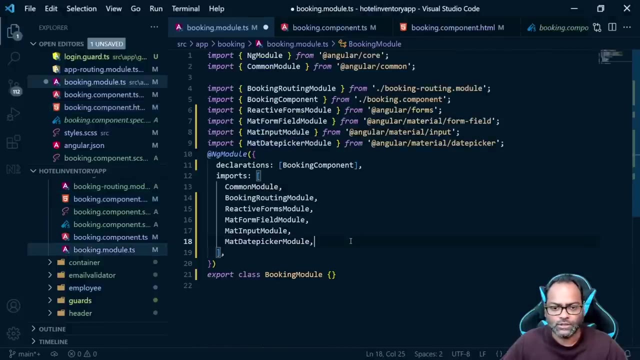 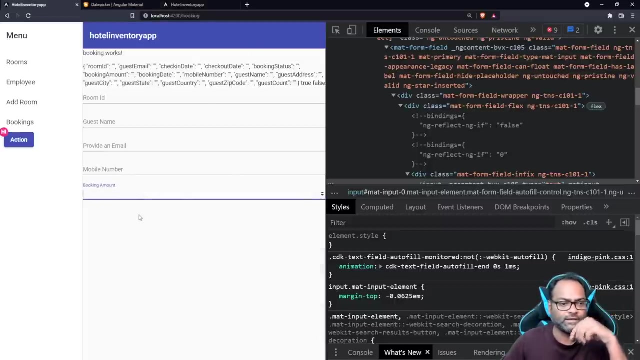 and let's format this and let's verify: okay, so it says, uh, mat date, because it is in the known property of input. so we added mat date picker module here and it is not saved. so you can see there was a white dot line, it was. it means it was not saved. and let's see the form now. 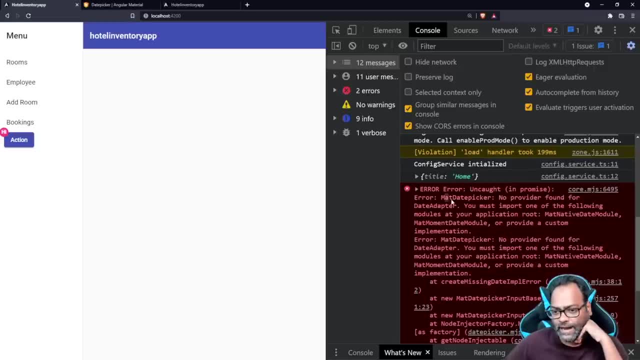 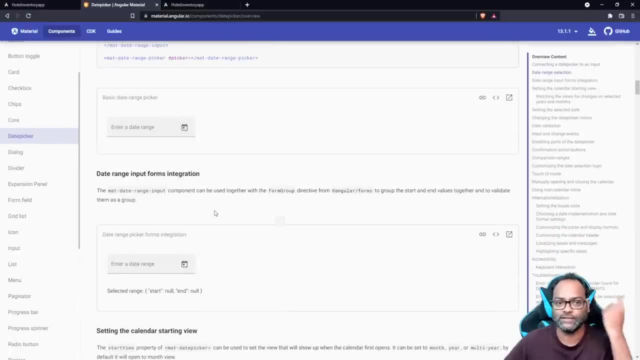 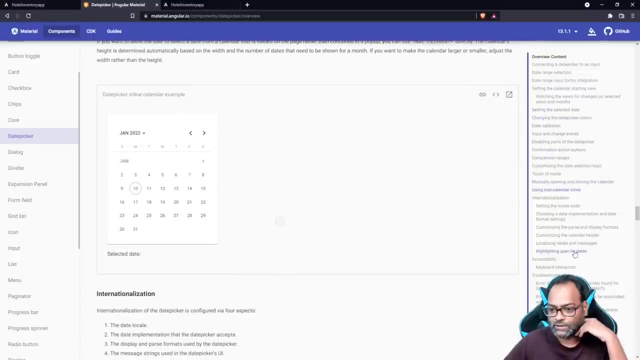 and there is again somewhere. okay, uh, so it says mat date picker: no provider found for date adapter. interesting, because, yes, we need to set something and it is already provided in the documentation. there is nothing. uh, this error is not wrong because we have. uh, this you can see here: internationalization. 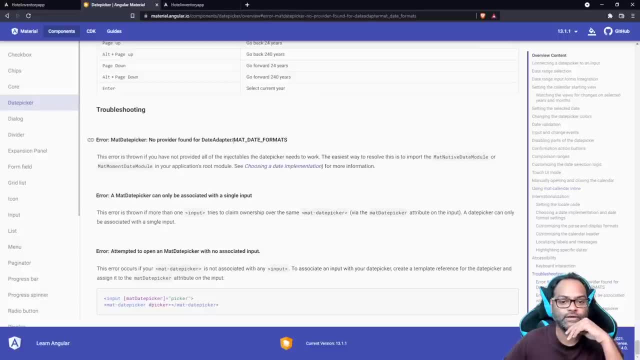 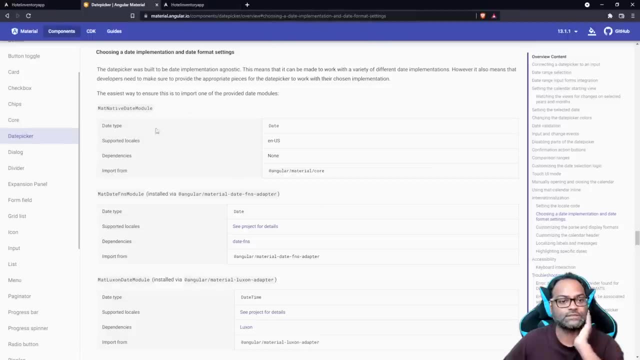 no, no provider for data adapter. so you can see it is already uh given in the documentation. so so it says no, not provided for all injectable date, because it's choosing a date implementation so you can use multiple uh date implementation which is available, and what we will do is: 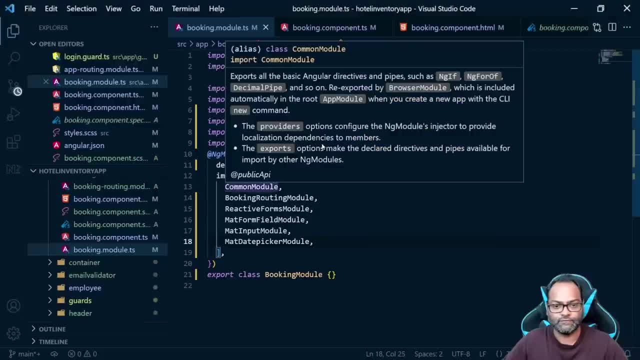 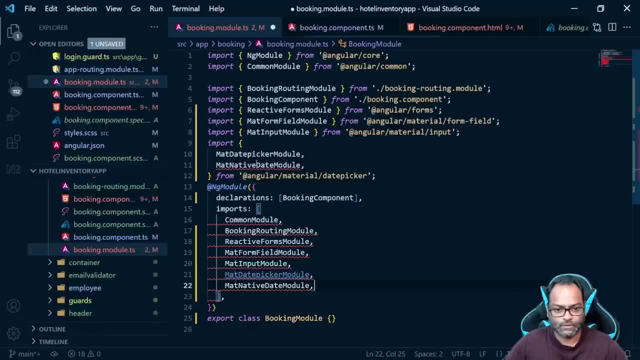 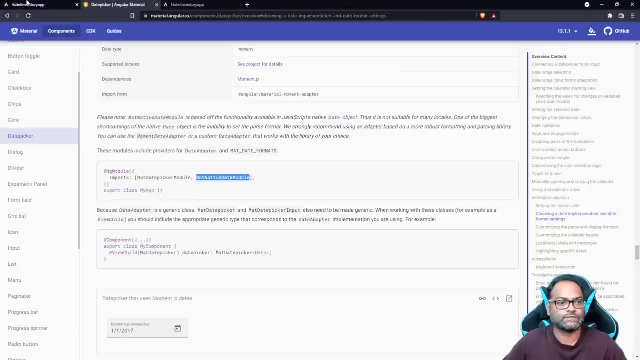 we will use native one, so i can just use mat, native date, this one module. okay, i think this is not part of this. so let's see from where it is it's part of over. let's see if it fixes our issue and bookings: yep, so you can see. uh, it doesn't. it has my. 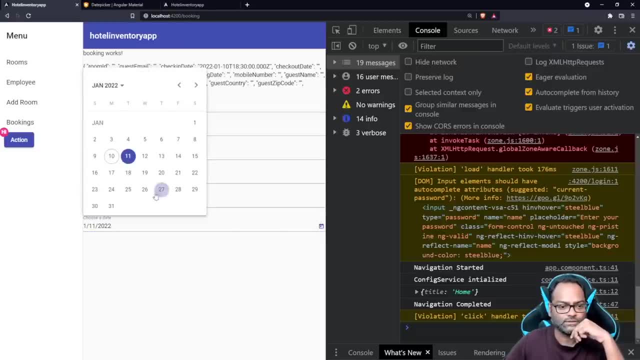 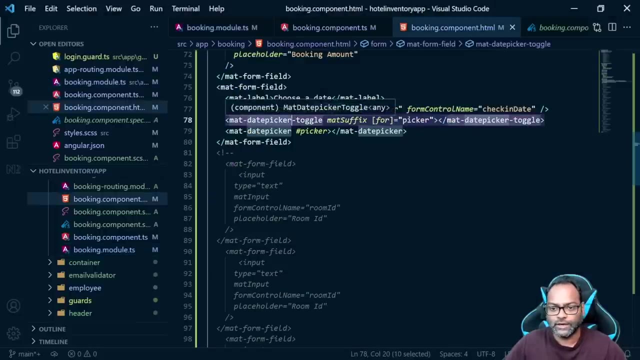 nice date picker and which you can choose and it shows you uh to our, allows you to access a calendar, right so? or date picker, so you have available. this shows a date you can. we can actually change, change this and say this is check-in date, right, so here now label will be changed to check-in date and you can see when you click on. 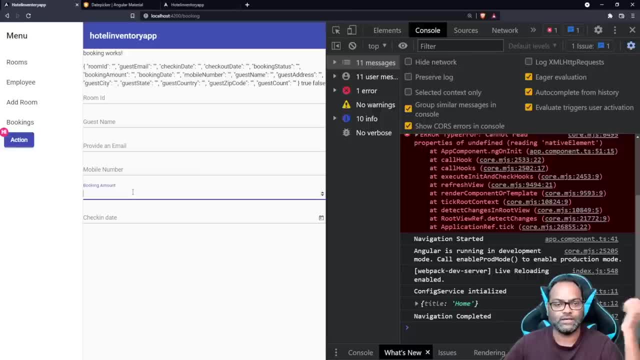 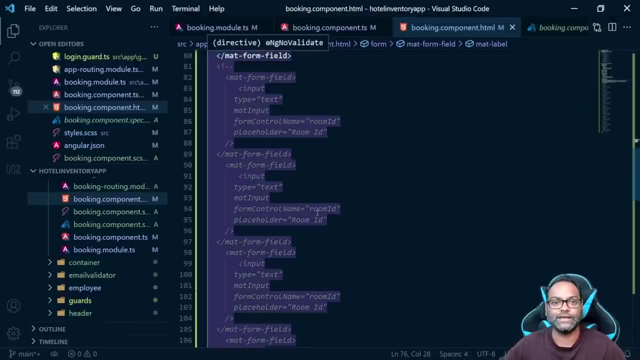 this. the label goes above it's. it's a mobile uh first approach, right? so whenever you are using material, it's a mobile first approach. so now we have check-in date check and all other controls which are available. so we also added and we also added in date become, so we can just go ahead and create all other controls. 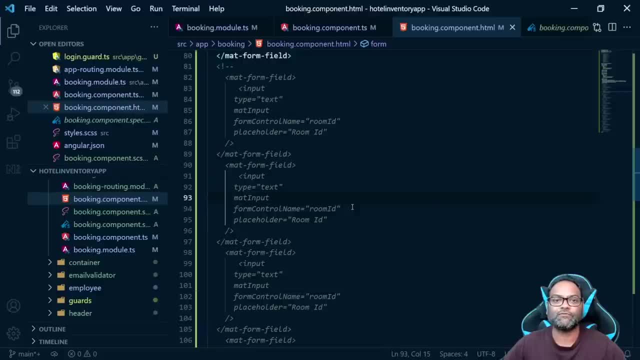 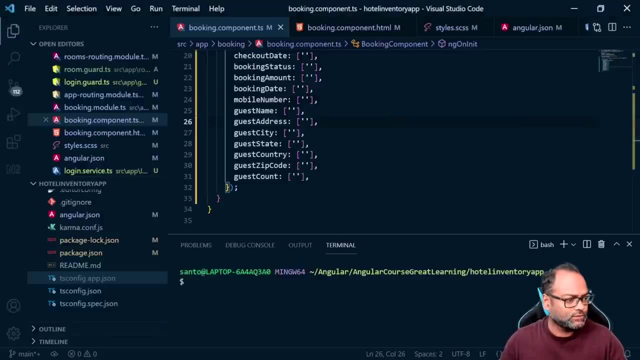 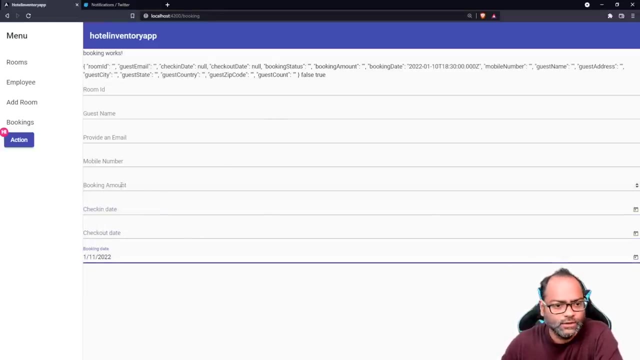 what we'll do is we'll add all the all other controls and then we'll see how our form behaves and then we'll add more controls. but i have created the forms. uh, i have created a few more fields. for example, we have not checked at checking date checkout, date booking, date booking amount, mobile number and email, and 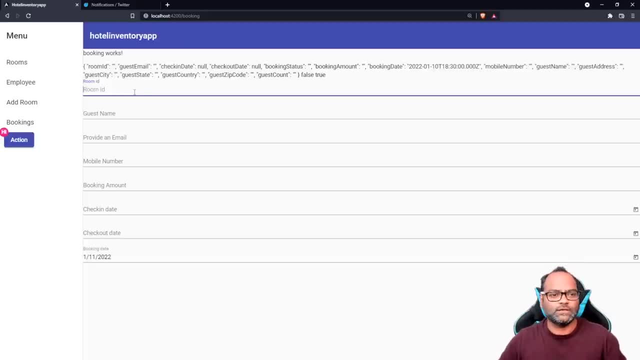 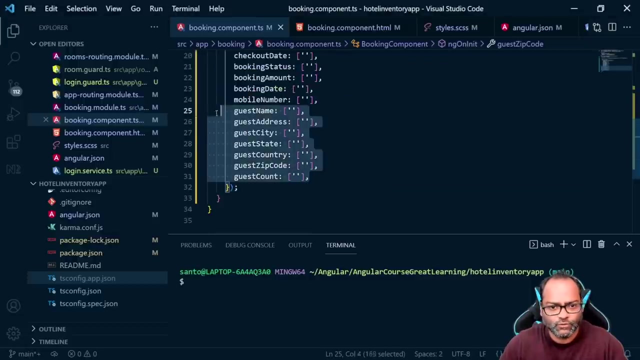 guest name and room id, which is right now our text box. but we will change it. we will do something like where we click on rooms and then book rooms and the id is actually retrieved from the url, which we already know how to do that. so here let's do something right. so we already have few more. 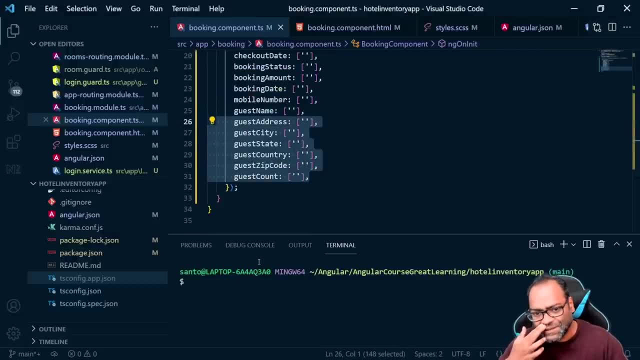 fields where we have address, city, state, country, zip code- and we'll talk about guest count later on. so what we will do is we will try to cover as much a scenario as possible here. so for the second step, we will add this address information in our second form. you, if you are wondering what is. 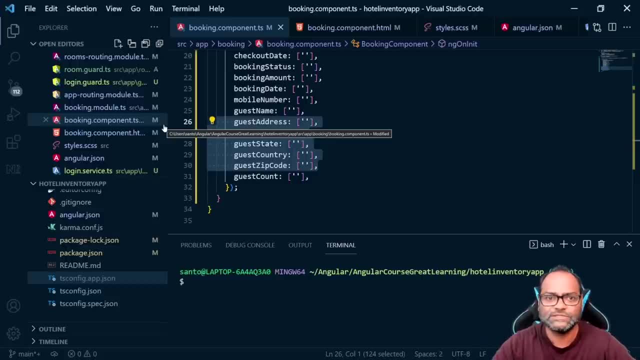 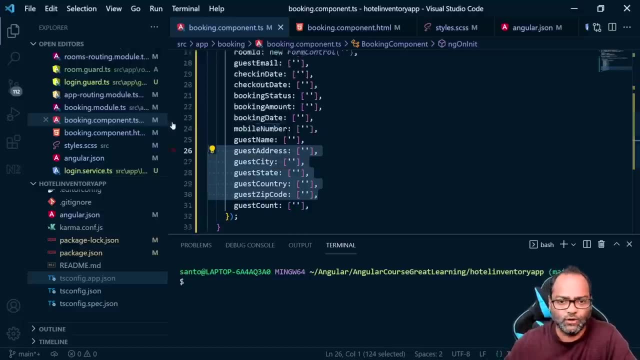 second form. so we will be. we'll do nesting form nesting, which is one feature which is available inside the angular forms which we can do. so this form, right now, as we know that this is a form, can have a nested form controls. so we will create another. 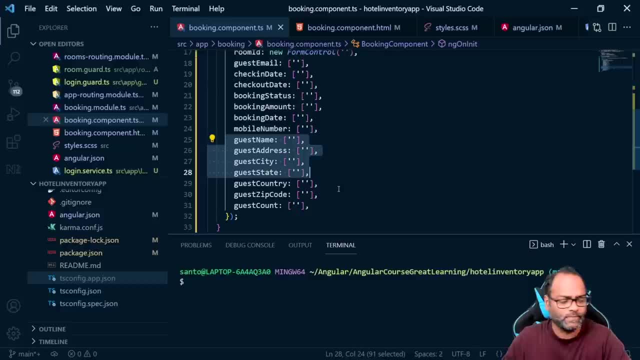 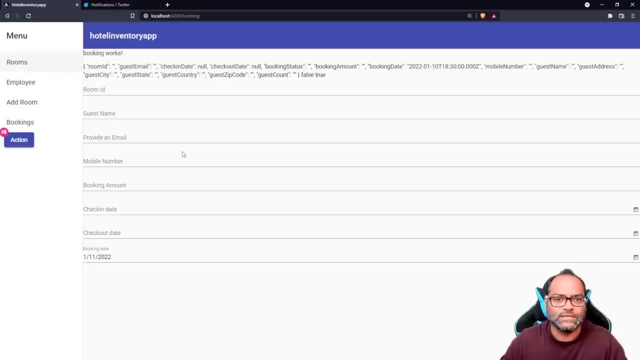 group of forms which we can do. so we will create another group of forms which we can do. so we will create another group form group inside this existing form. but before that, let's go ahead and talk about few more things. let's go ahead and see how to submit your form. 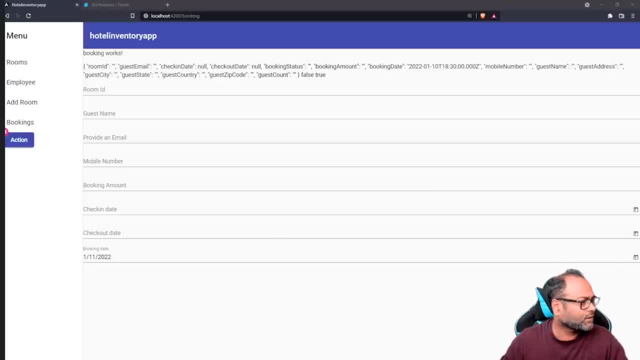 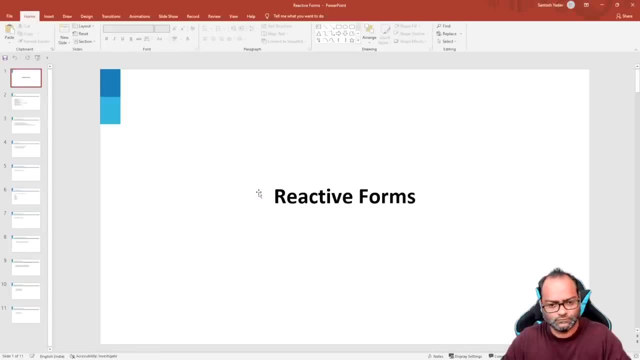 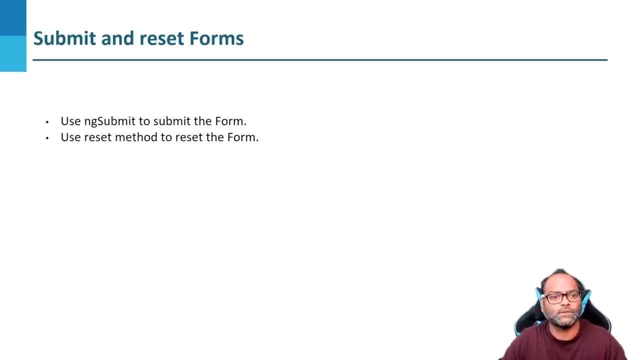 inside this existing form. but before that, let's go ahead and see how to submit your form. so we will see how we can submit the format and then we'll be back with some few more things, for example, how to add this, this nested control, nested form control- then we'll. 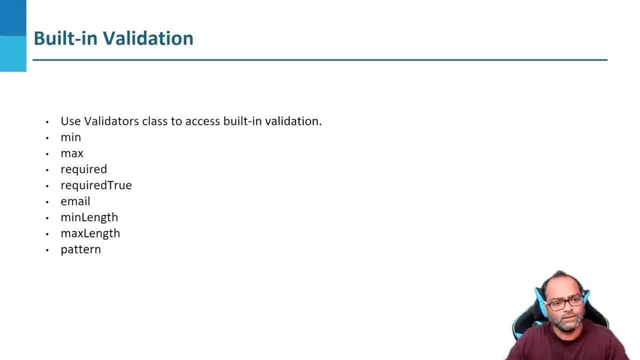 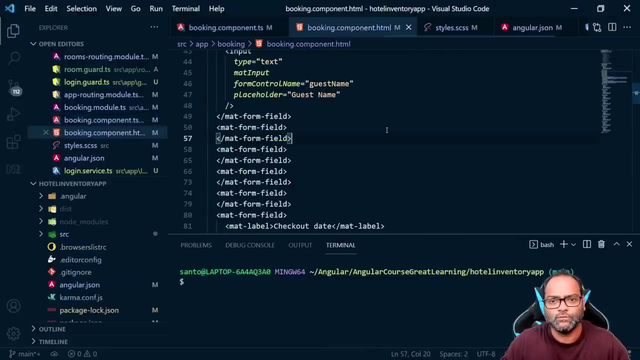 to go ahead and see how to submit the form, about how to to add this new one. so i'm using the example controls dynamically and then we'll talk about built-in validators. so, uh, let's go back to booking componenthtml and to submit the form. we have to use the same. 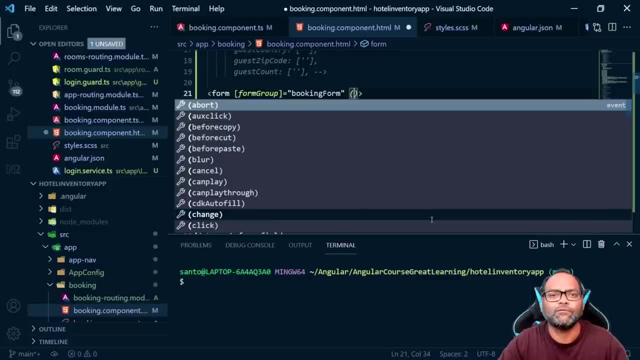 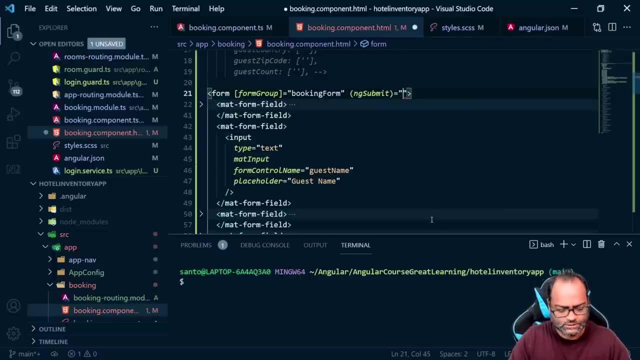 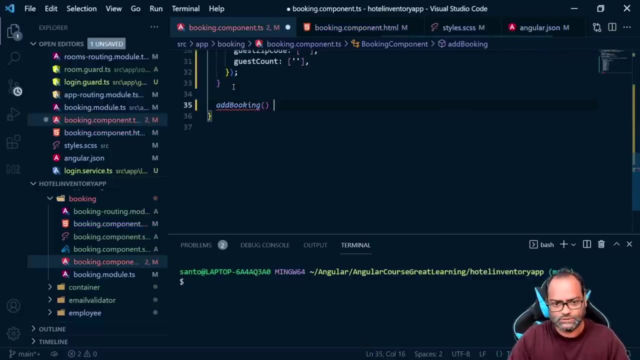 uh event which we had used earlier, if you remember, in template driven form. we used ng submit. so we'll say, okay, this is something we submit equals to, and i'll say: this is add uh again, right, so here, uh, let's see, this is uh, and then we'll do consolelog to see what is the value which we're. 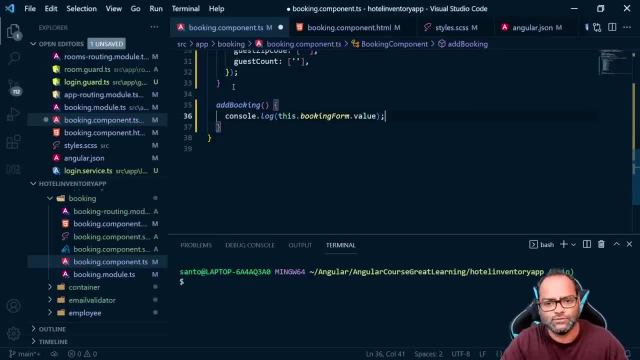 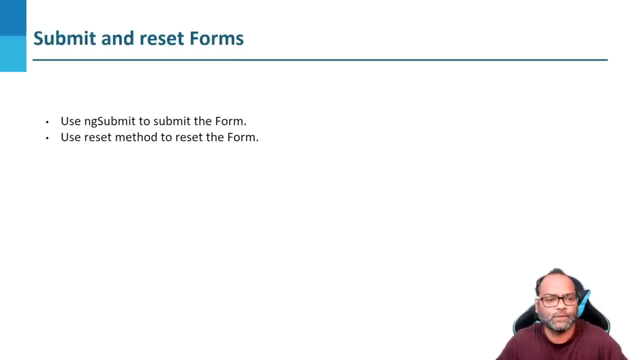 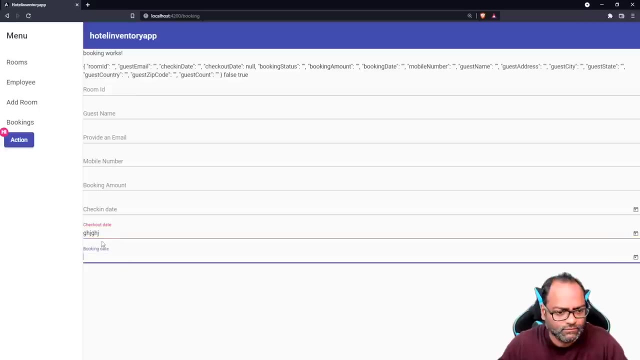 getting. so if, uh, you might be wondering how to get this values right now, so you can do something called this dot booking, dot booking form, dot value, and let's verify it right. so one thing which i want to show you here is: let's say, if i enter a, 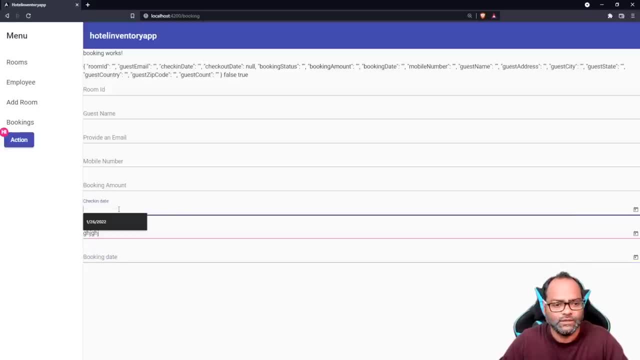 wrong format here, right? so, as this is already date picker, i mean, you can see the validation error is already there and this is how actually angular material shows validation errors: it it becomes red. so just to let you know in case. so, uh, let's go ahead and see. 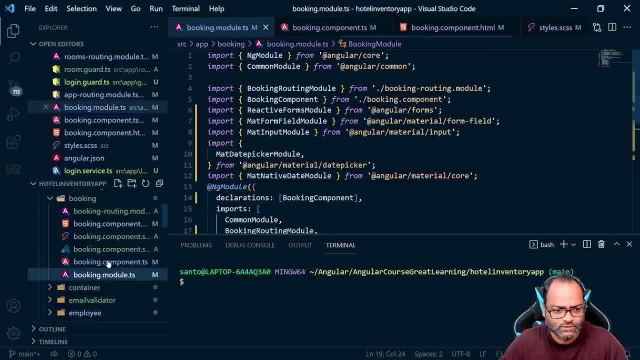 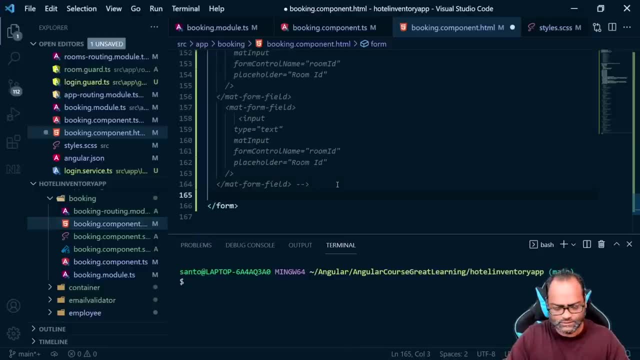 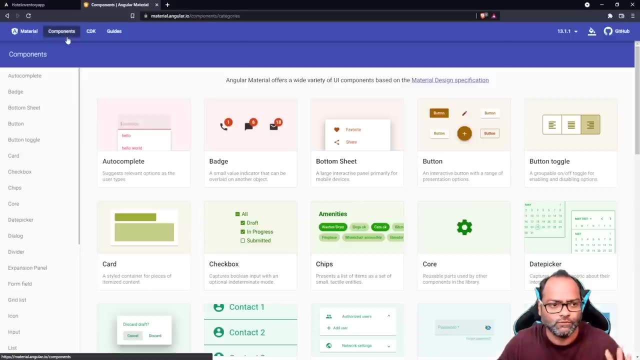 so before we can submit, we need a button as well. so let's add a button, which we missed, and we will be using angular material button now, and to do that let's go to material docs right. so on materialangulario, we have a lot of components. there is a button. 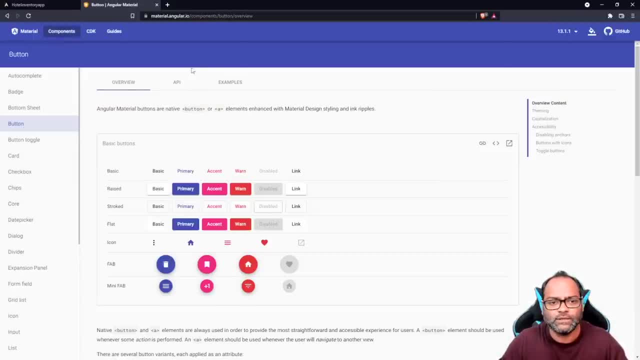 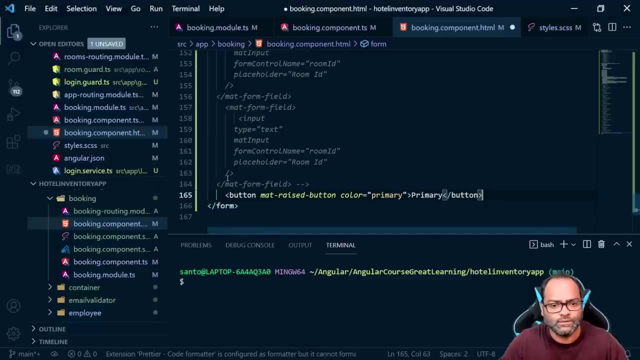 component as well, and we will use this primary button. so i can, we can- just go to example and see the code and let's copy this primary button and put it in the here, which i will put inside another div. and as we are using material button, uh, we need to add: 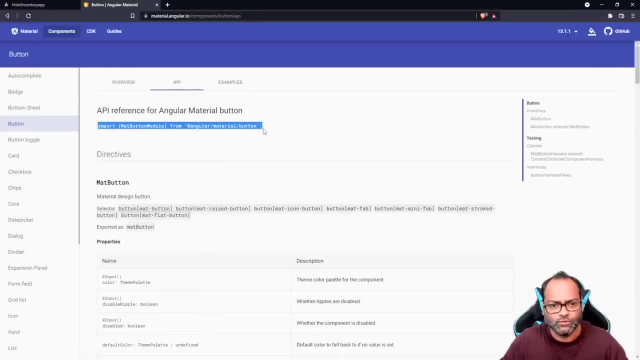 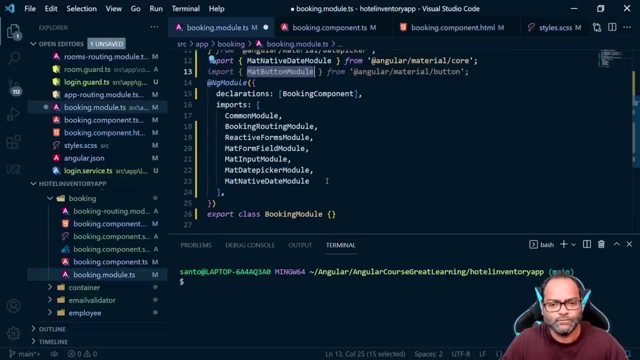 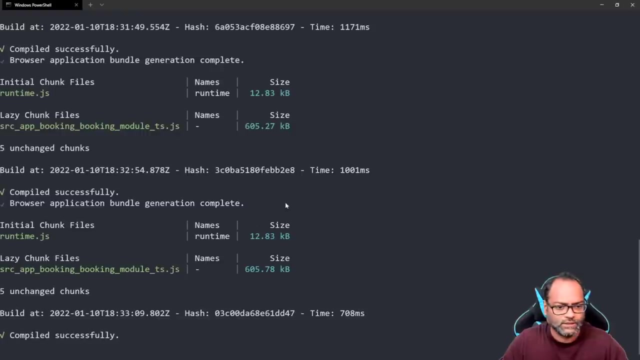 also the api. so we will say import mat button module, which right now is used inside this one booking module. in case i'm using it, uh, in other forms you can also add it to app module. let's go and see. uh, this compilation is done, let's see the form and we have this button available here. so 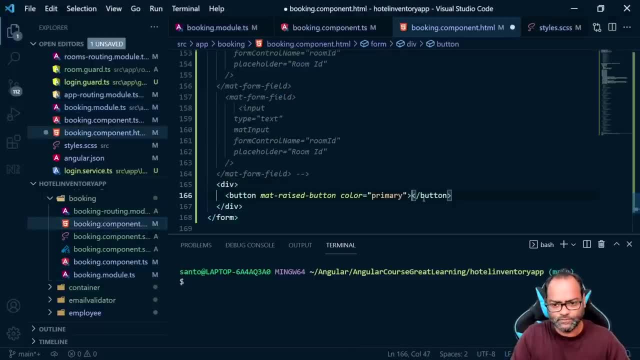 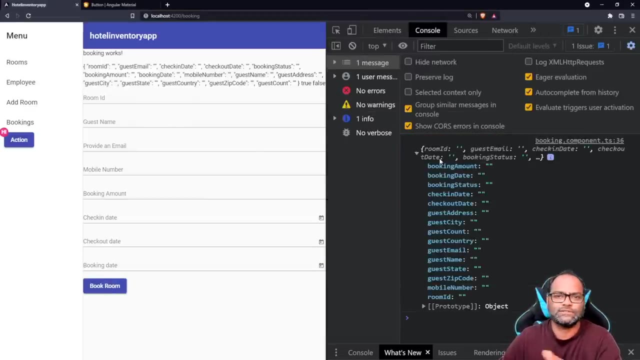 everything works, even the css works, and we'll say book room. let's go ahead and see in console, let's clear everything. let's click on book room and you can see. you have all the properties. right now it's empty because we have not submitted anything. let's click uh, let's provide the room number, guest name. 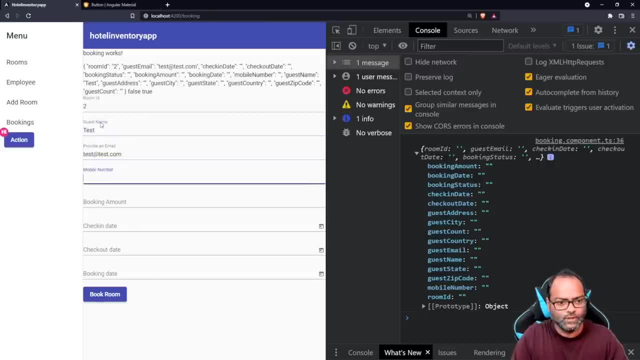 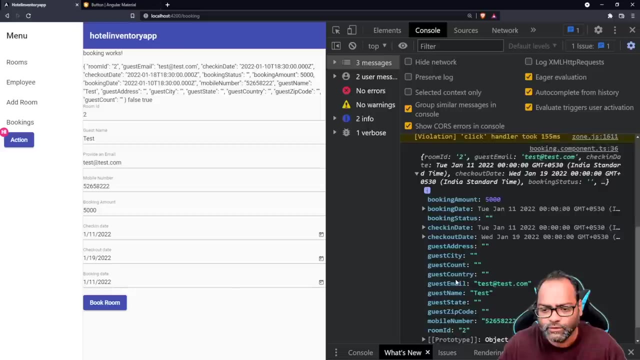 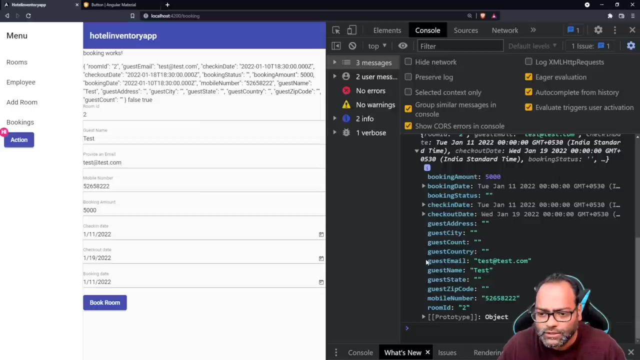 uh, provide an email, mobile number, booking amount and then we'll have check-in date, checkout date and booking date book room and you can see you have all the information which you have submitted. so you have booking amount, you have booking date, book check-in date, check-in, checkout date. this would be guest name, email, uh mobile number and. 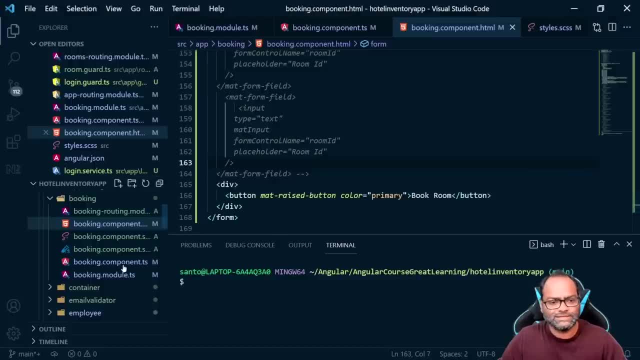 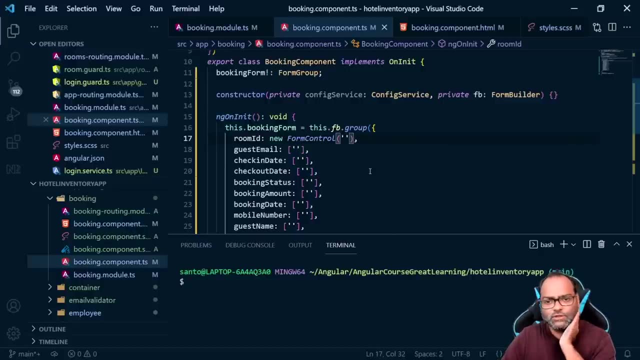 room id. so everything is available, but there is a catch. what in case? uh, so let me show you what. what, uh, what is the catch here? so here you can also do something like this, so you can actually say: uh, that, okay, your default value is two and that, and, uh, you want this. 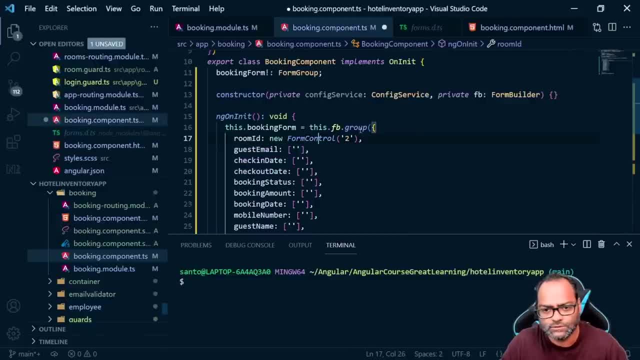 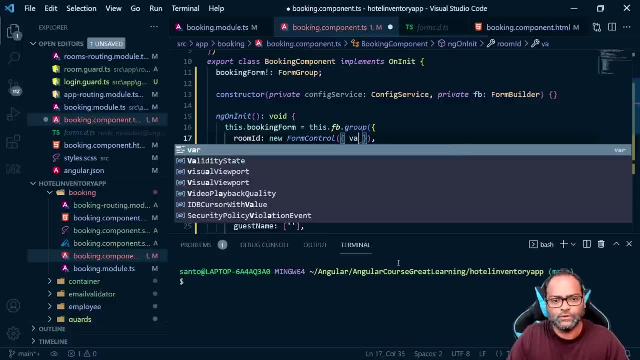 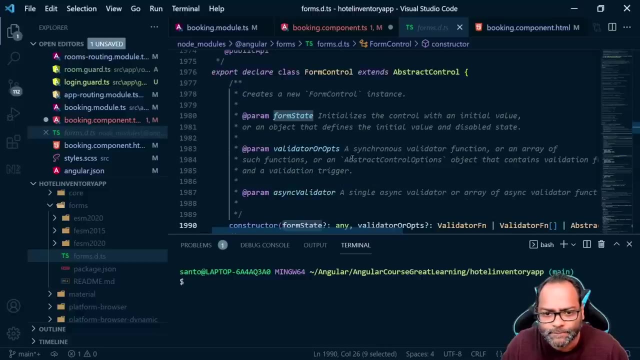 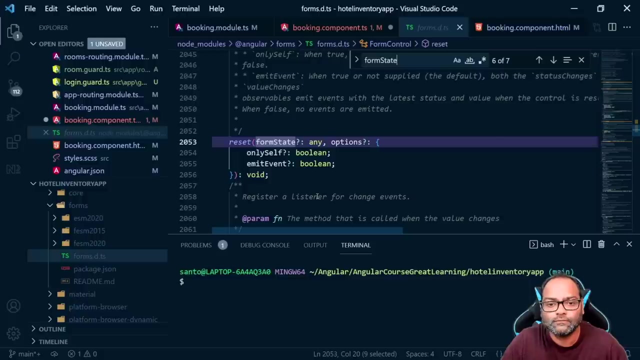 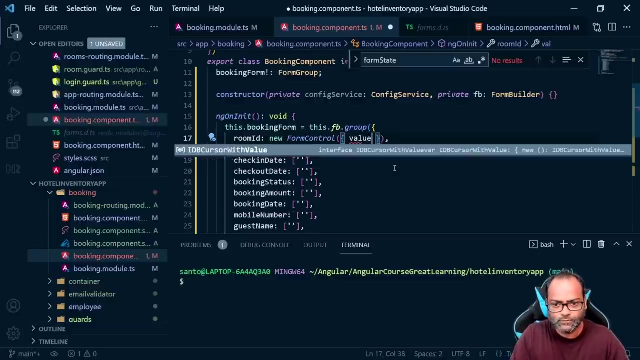 let's see the api. so forms right. okay, so so you can submit uh form state which looks like this: um, this is the default value of your form. let's see what happens here. we don't have any typings here, so that's what the problem is, and 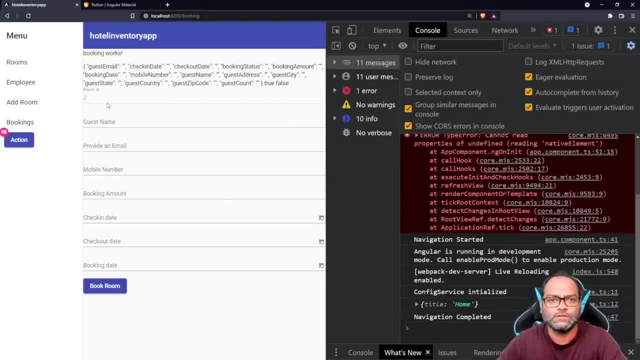 you can set value and a disabled state. let's see. let's see what happens in this case. so your form control will be disabled. so you can see the value 2 is available here, but the state of this control is disabled. so or you can- i mean you cannot- type anything here, so it won't allow you. 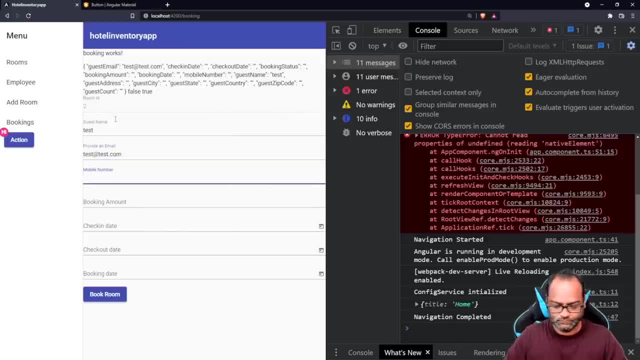 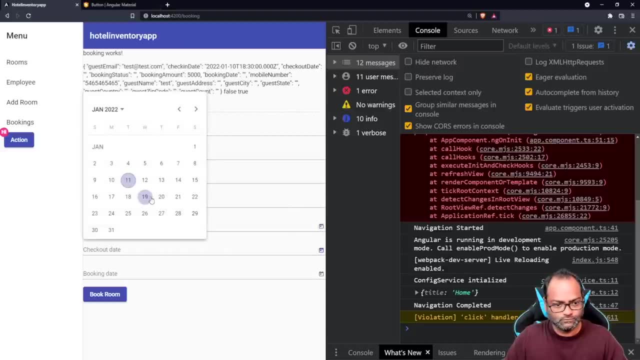 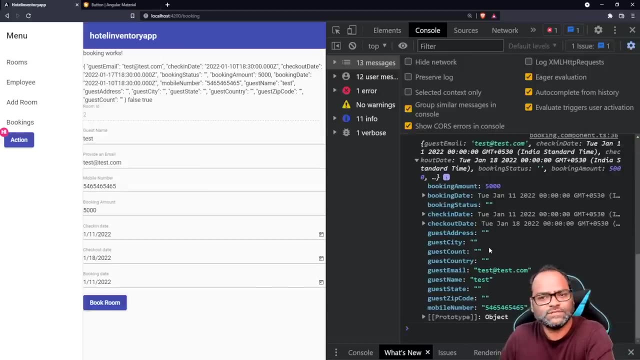 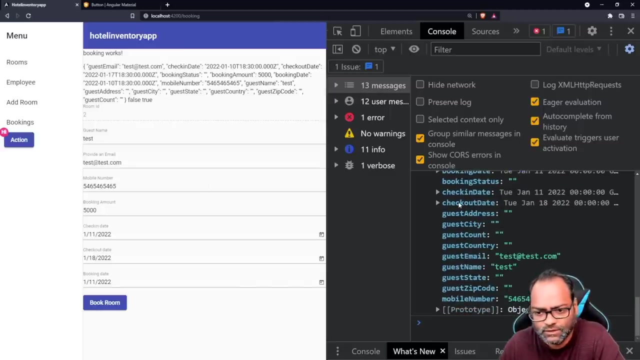 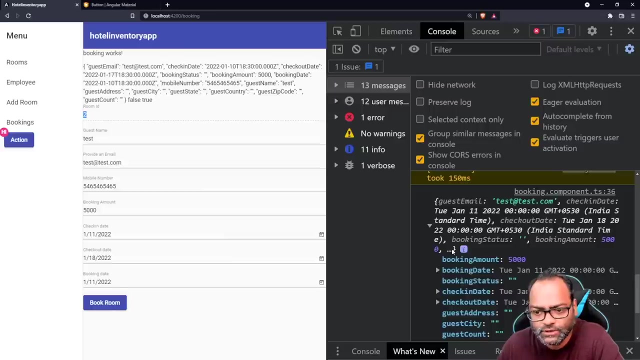 and see the catch. okay, so can you see something is missing here. let's zoom in any property which you think is missing. yes, the answer is room ID. you cannot see room ID available anywhere, even in the object. even it's in form. we are not able to get this particular value. 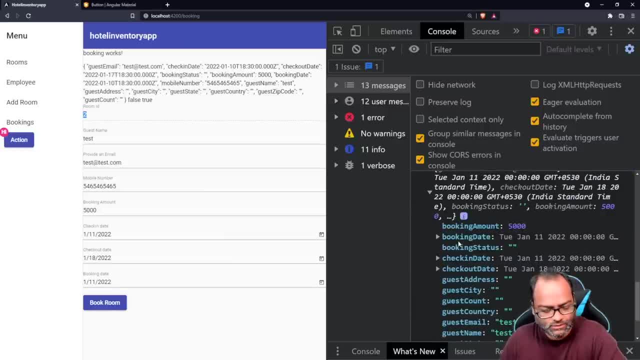 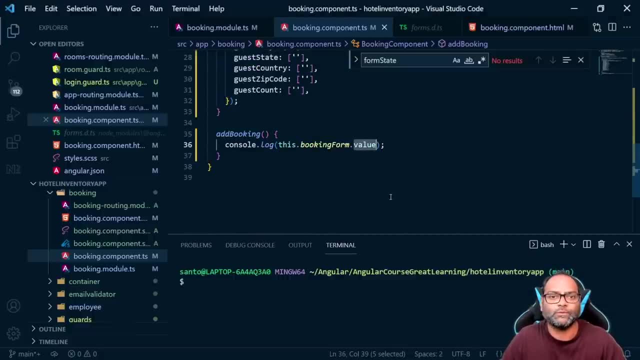 which was available earlier. this is one thing which is not available when we try to access the value dot value property. so try to use another property of form which is known as get raw value. so get raw value will also give you the values of the control which are in disabled. 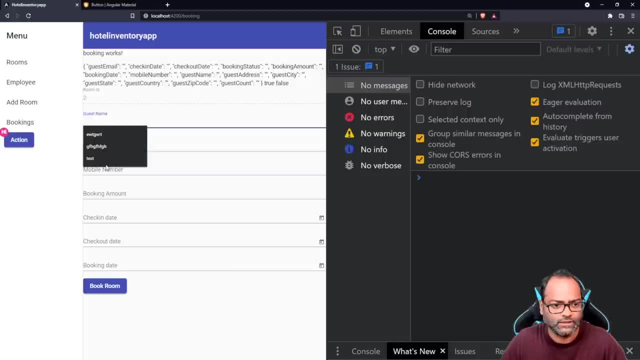 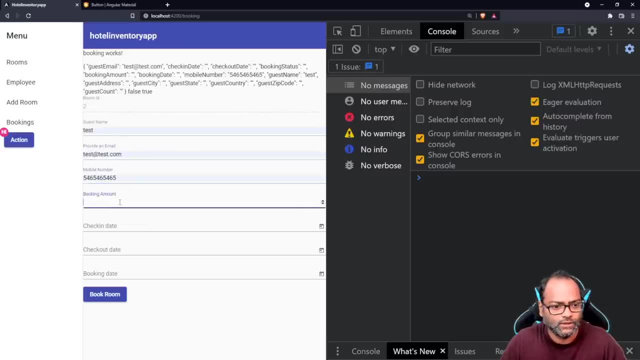 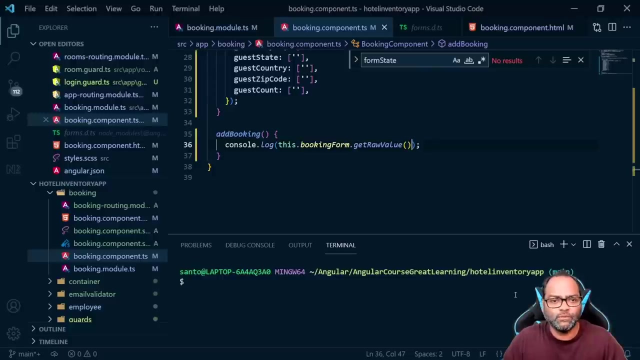 state. so let's clear it. let's enter the email mobile booking amount, so checking date, checkout date and booking date- and click on book room and now you can see room ID is available as well. so remember when you submit this submit form and you want to get the data out of that. 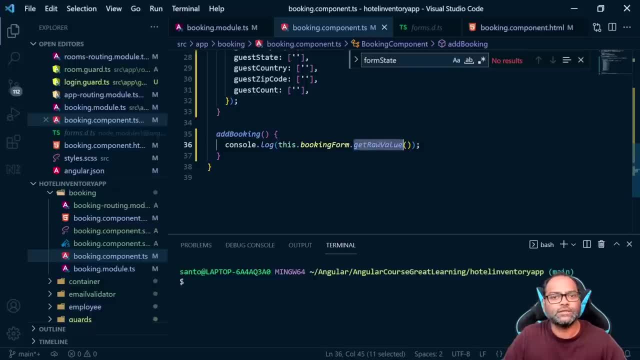 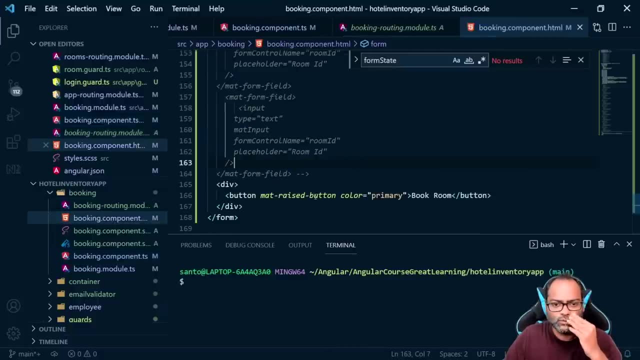 particular form try to rely. So this is one thing which we wanted to show you. now let's move on and let's add the next part. as we said, we will be nesting the form, what we mean by that. so here you can see I have a lot of. 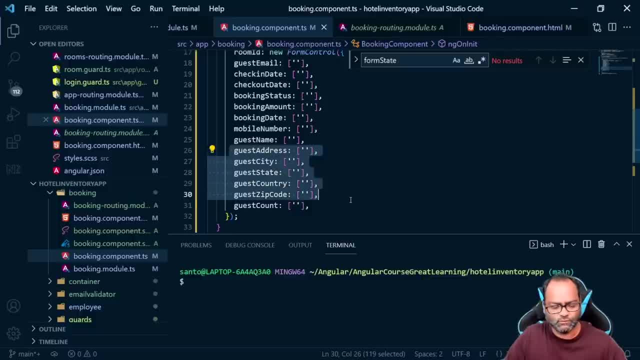 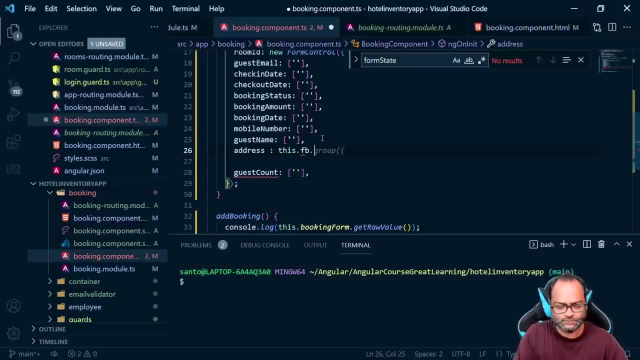 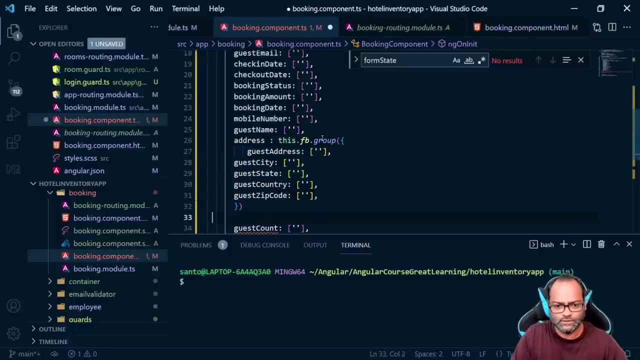 controls, right. so what we want to do is we want to do something like this. so we want to have another form control which says address, and then this address contains the values, or you can say the form controls, and so this is how we want it, our form, to look like. so there will be an address object which will hold. 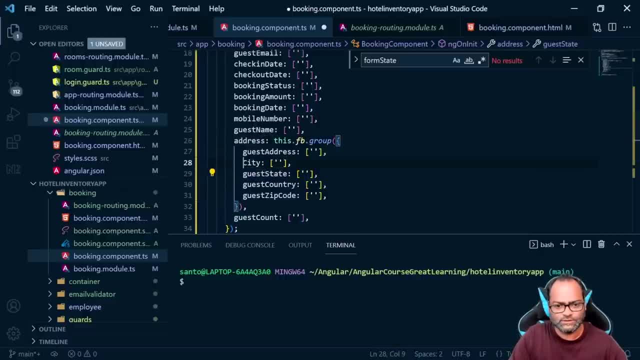 I can say: this is: let's remove this guest, right. so we can say: okay, this is state, country, zip code. and here we can actually break this into two address line one, For example, let's say address line 3 address. We can see that this address has some things written here. 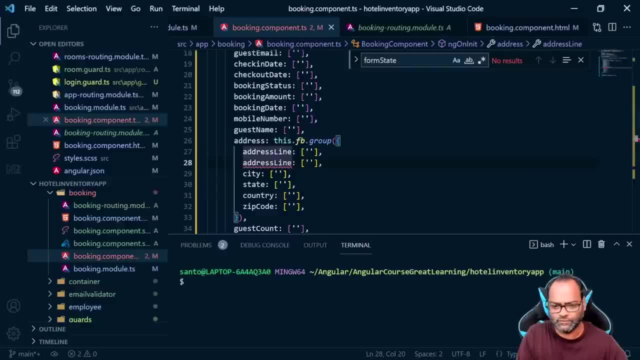 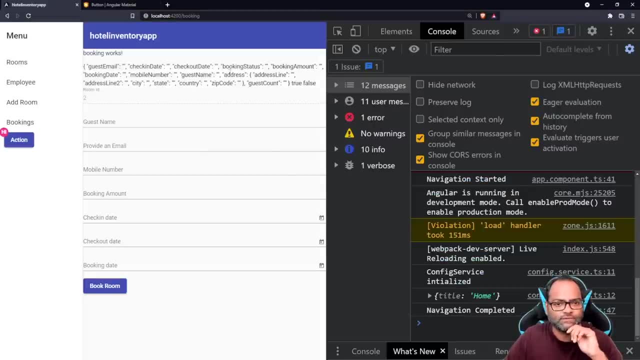 And we want them can collect some data in this form, Because most of the, I think, definitely just explain Texas that this line three, So we aren't this one. good, look like this and let's verify this. forms created in such a way we can see address and yes, it is right, so you have that. this, and then at risk contains all the subjects, etc. 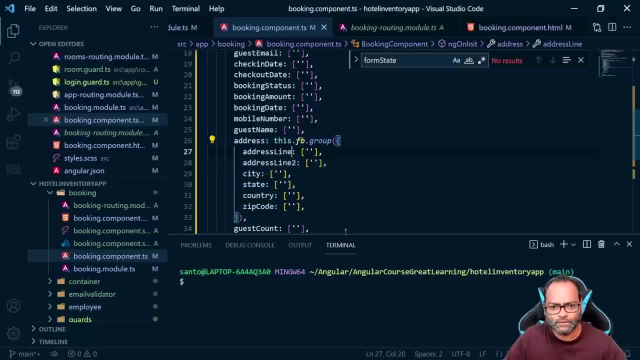 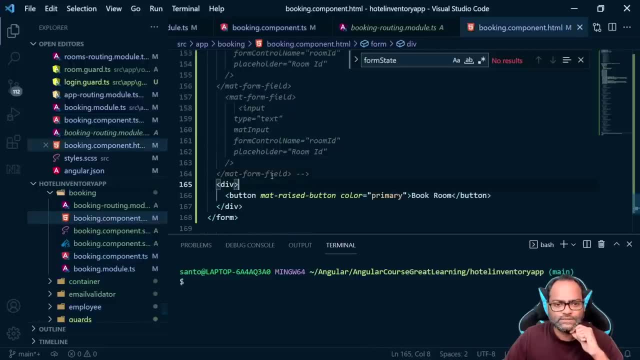 I just line, I just line, I just line two cities, state, country and zip code. Let's see, And don't be Harry is lie. Okay, This is an address lined two: city, state, country and zip code to render this particular form on our UI right now. So the first thing which we need is- I'm going to 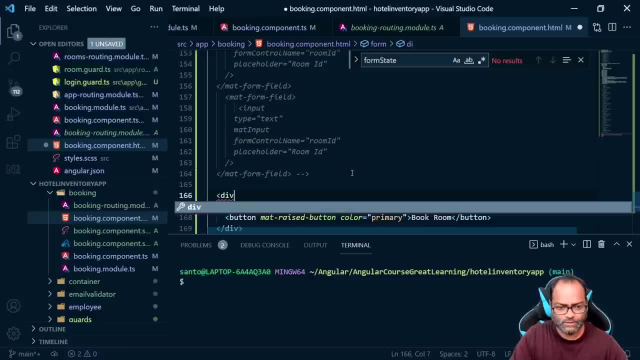 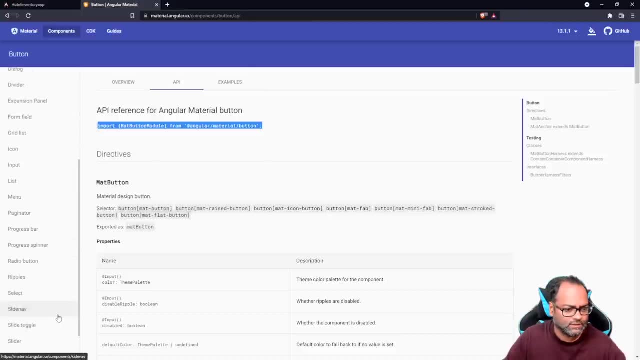 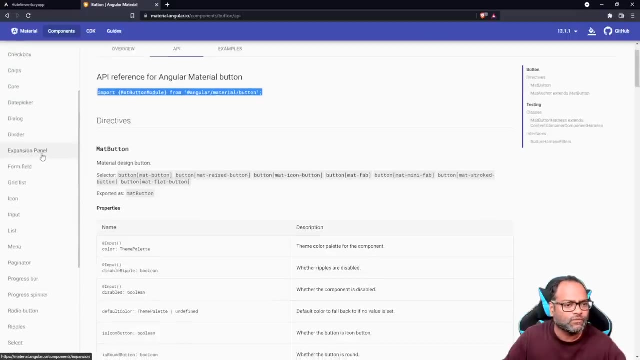 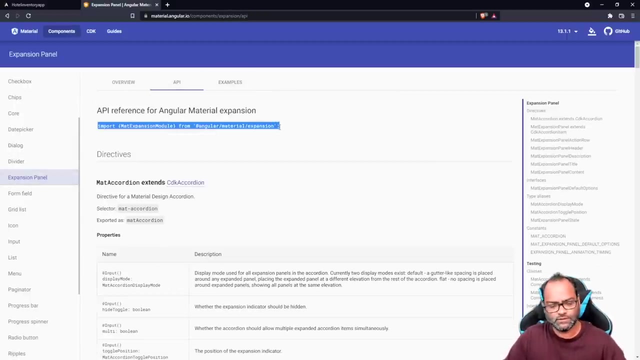 wrap it inside a div and let's add accordion control. So here we have something known as- let's see expansion panel. So angular material contains something known as expansion panel which we can use. So we will be using this API and let's go ahead and add this. 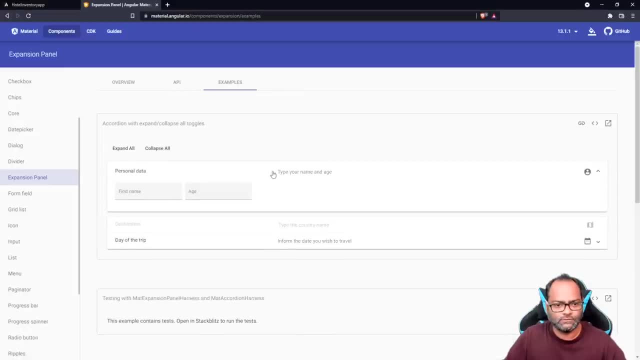 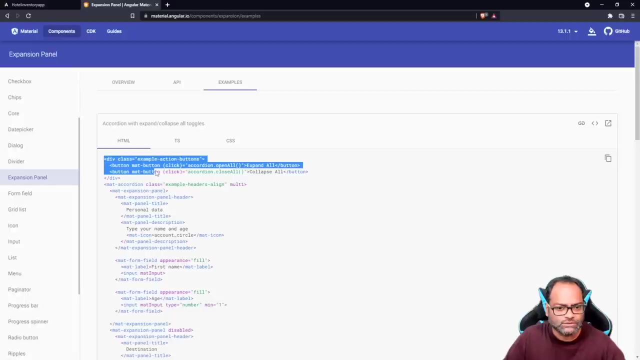 Right, so we added met expansion panel and now we want something like this: right, so where we have, we can click and it will just open all the addresses which we have. So let's see the code, and this is two buttons and these are the form controls. right, So we will. 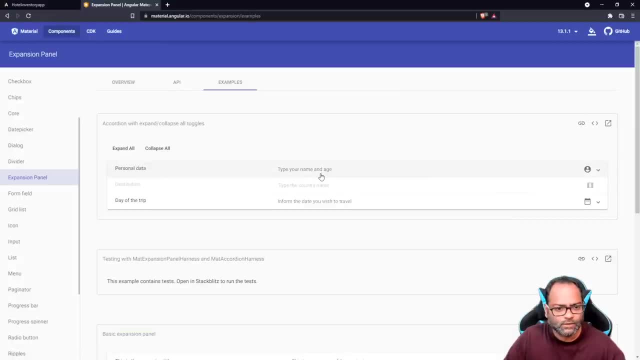 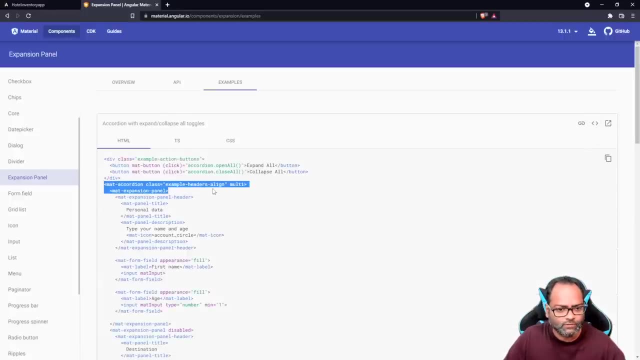 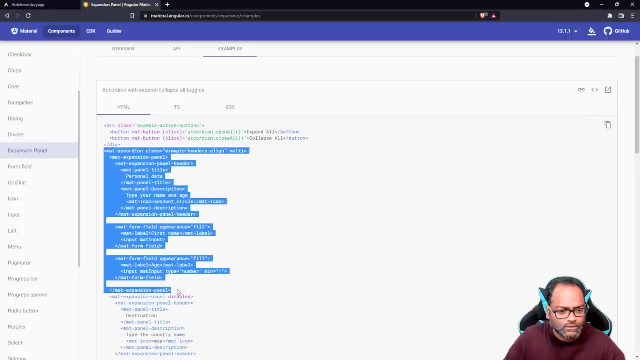 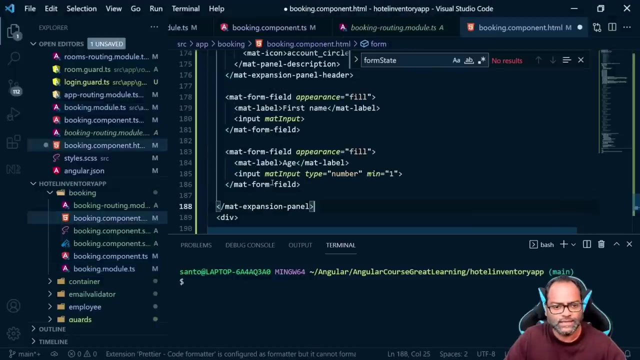 okay, let's see. okay, there is. okay, this is the expand and collapse button. we just don't need that anyways. So we need from here, mat expansion panel accordion. and let's see, I'll just put it as it is and we'll close the accordion and we are also using mat icon. 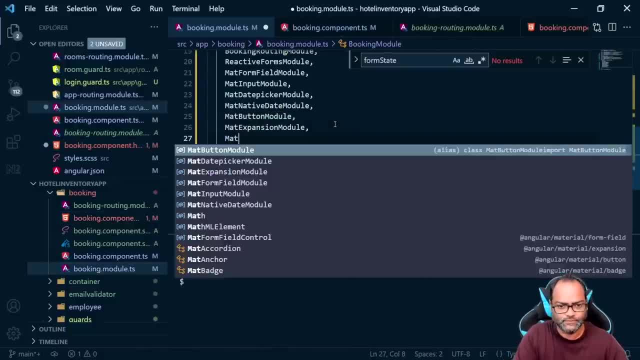 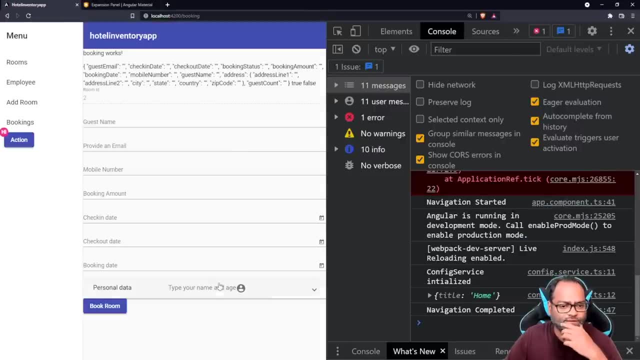 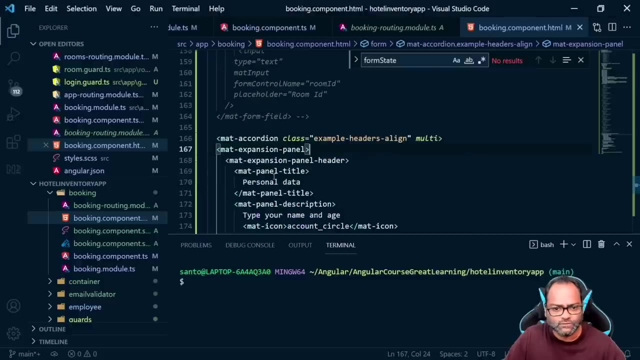 so let's add that as well. So mat icon module, And this is it. Let's see, let's see how our form looks like right now. So you have this personal data, so we let's, let's replace all this object right now, right away. So we will say: this is: 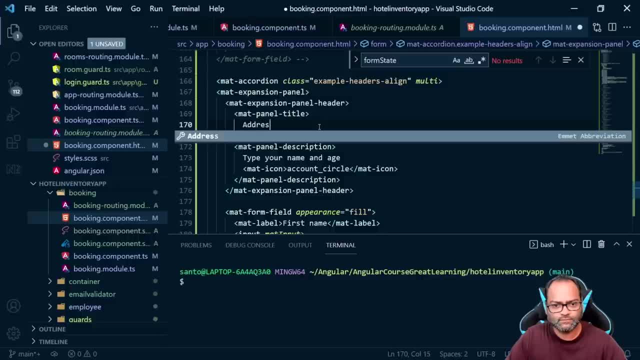 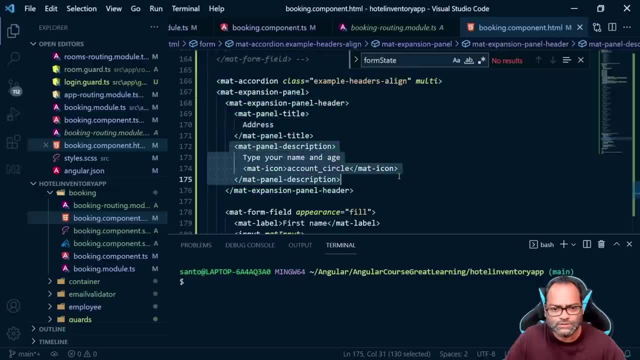 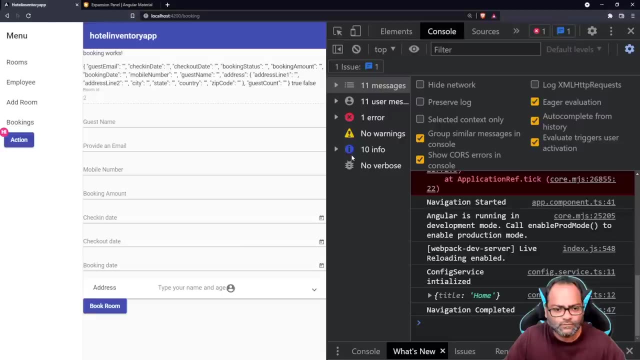 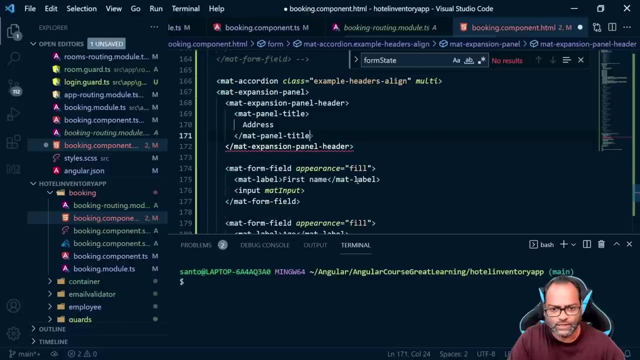 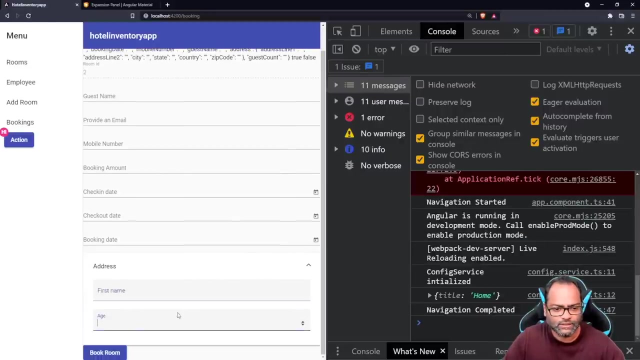 address, and here we want to add matpanel description. we'll remove this. or, and let's remove this matpanel description, so we just have a title right. so cool, sounds, looks good, and then we will add the other properties inside this. so let's start doing that and we will take. 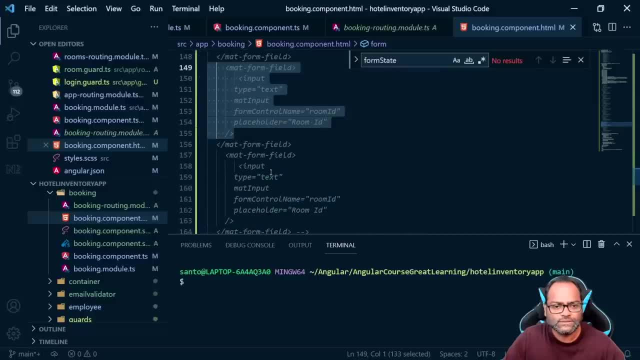 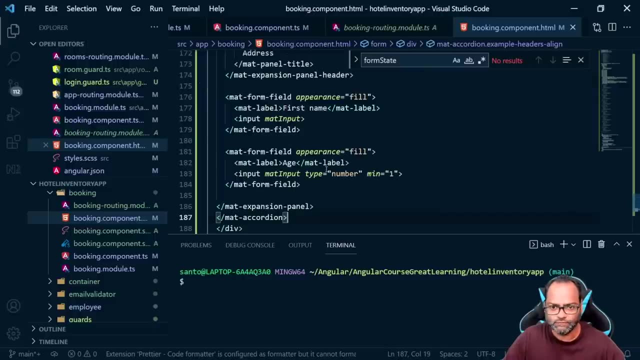 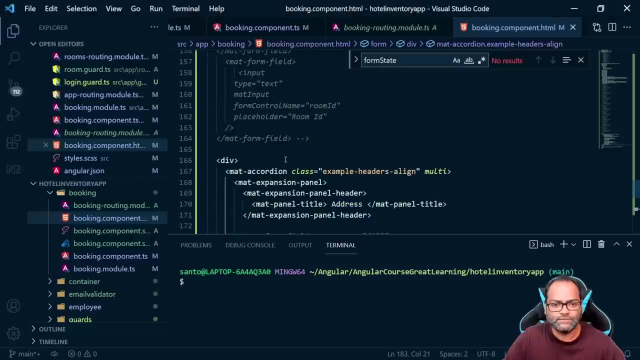 let's see where is the div gone, because that's really important here. okay, so i'll move this mat accordion inside the div. i'll just tell you why i did this. let's first create the form. okay, so we have this address information available here and let's copy this matform field. 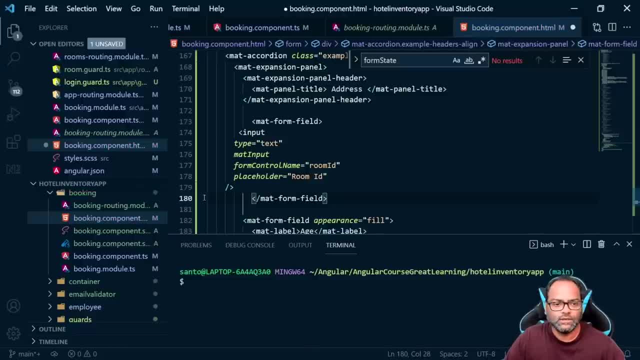 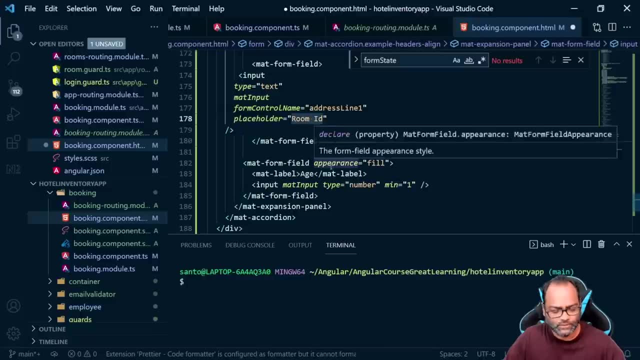 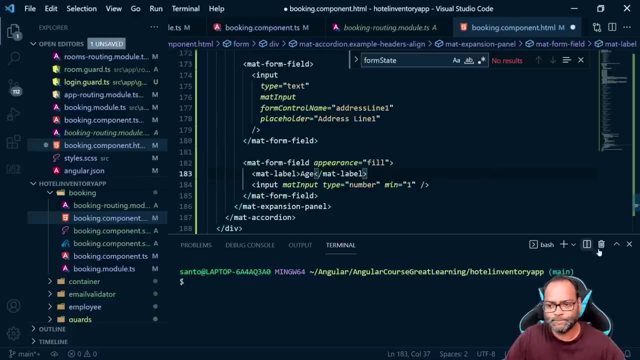 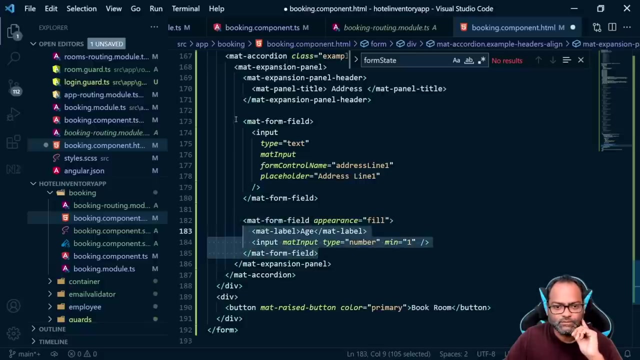 i think the closing of is missing and let's try to use this address line one as form control name here and placeholder is address line one, so let's format it again, okay. so what we have done is right now, this matform field anyways does not mix. right now it's not used, but this is the one which we added right now. so we are saying: 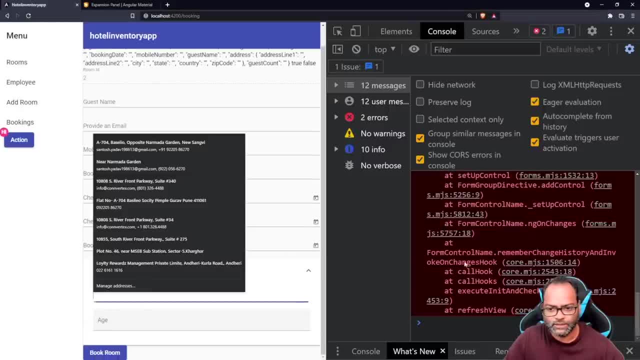 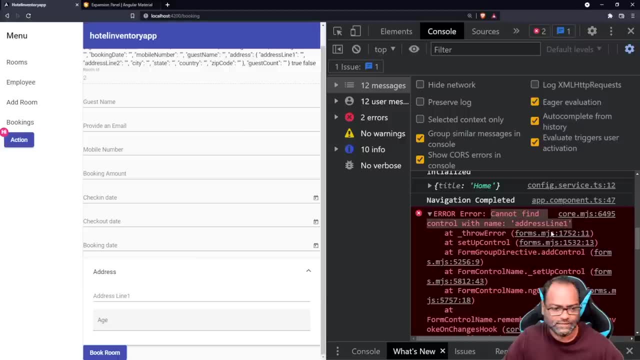 at this address line one is the form control we are looking at. but here let's see something which is available here. cannot find control with name address line one, and you might be wondering. i mean, this control is available here, but can you see if i type a name? 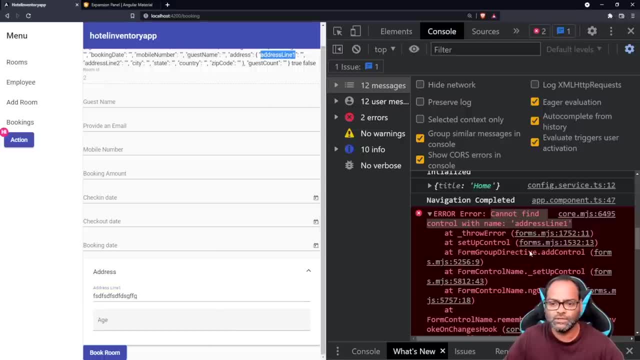 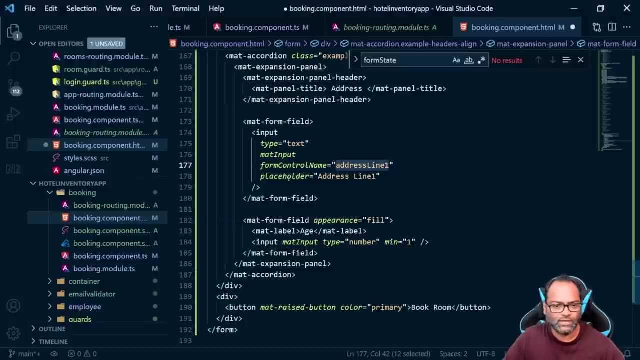 if thing here, it is not getting reflected into this particular control and there is also an error which says i cannot find this control with address line one. but you might be wondering, okay, i mean this particular control does exist here, but how it is not available. so this is where 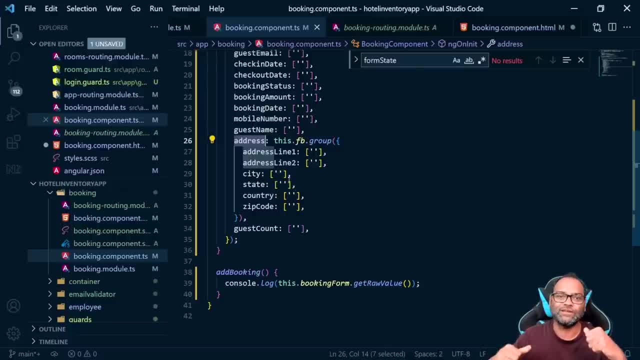 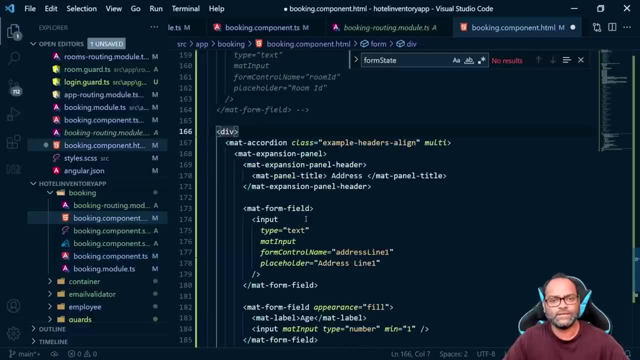 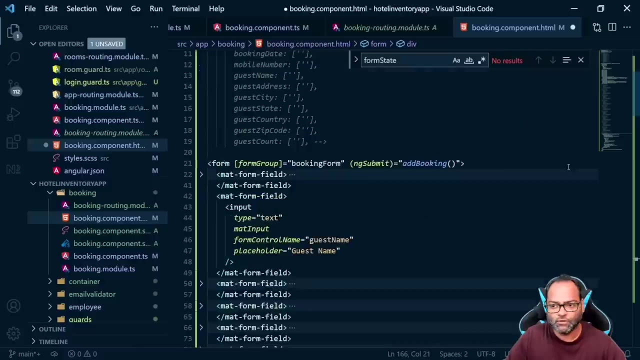 uh, we have to understand one thing: this is another form within a form, so to access this particular controls, the first thing which we have to do- is that's the reason i place this div- you have to use form group name. remember, we have already used form group here and there can be only one form group. 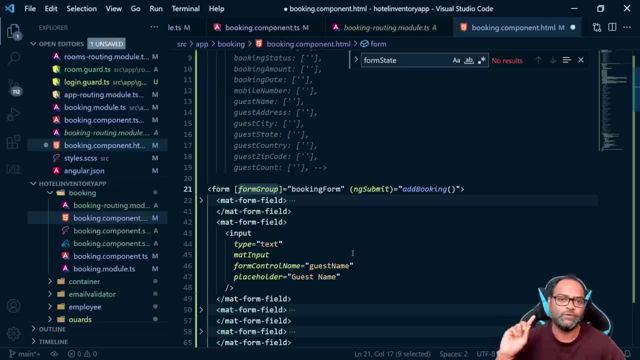 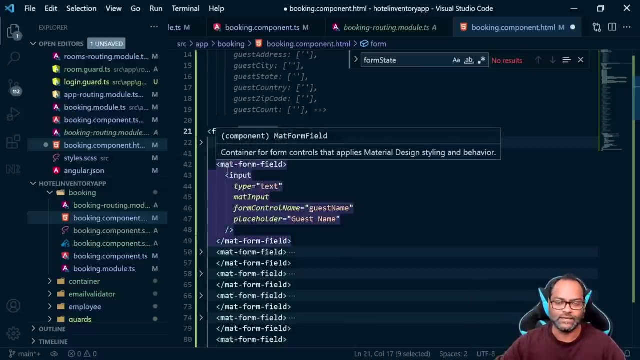 on a single. uh sorry, there can be only one form group on a page, so this form group is available now. anything which you want to add inside a form can be nested form and another form, right? so it's okay, i can create another form using this fbgroup and that can be another form altogether. 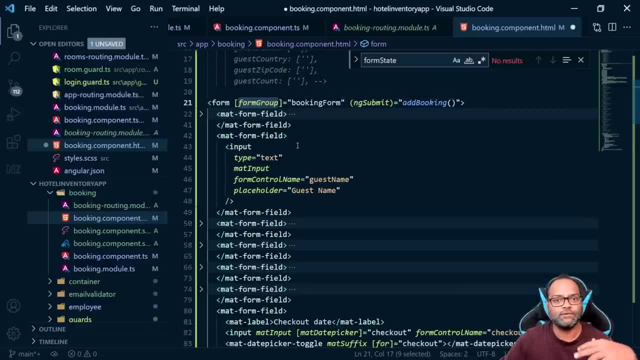 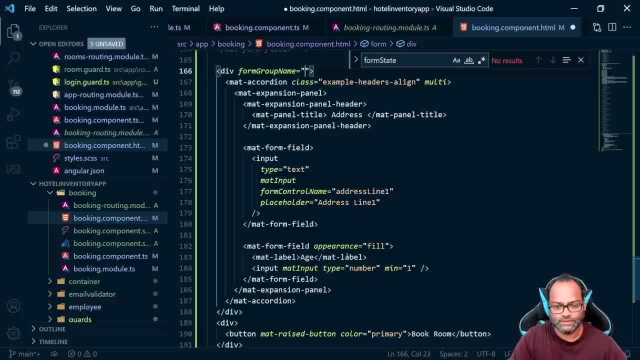 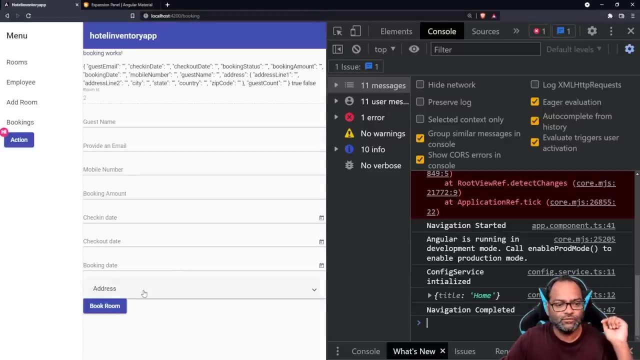 but if i'm adding it inside the form same form, it can be form group name now. so we'll say, okay, this form group name is equals to address and we are saying any control which will be available inside this particular div will be related to the address. and you can see the error is gone. 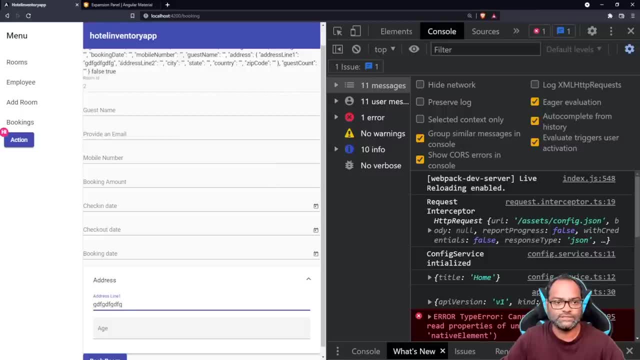 you will not see any error. let's address: enter the address and you can see it is getting applied to this address line 1 property. similarly, we can add address line to city, state, country and zip code, all those controls. so now your form looks little bit better, right, i mean, it's it. 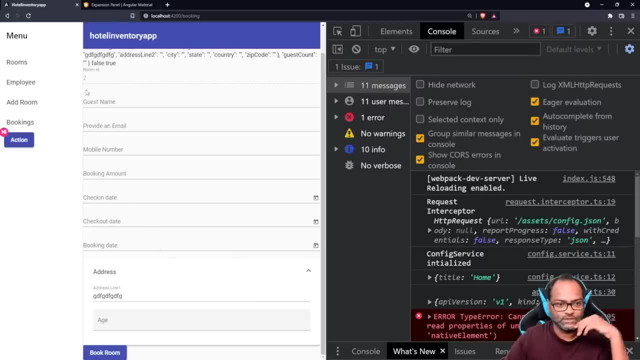 looks much better. i would say we can actually also move this section, the entire section, into another accordion or expansion panel and it will look really nice. so we, we will have list information displayed while submitting the form. so, uh, what we will do is we will add all these controls. uh, let's. 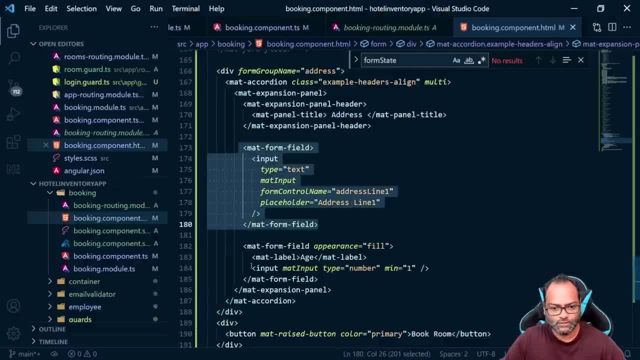 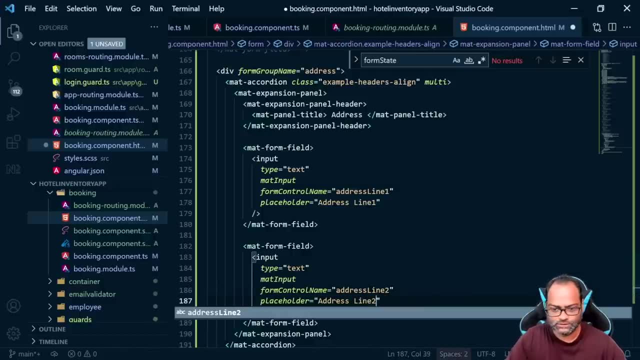 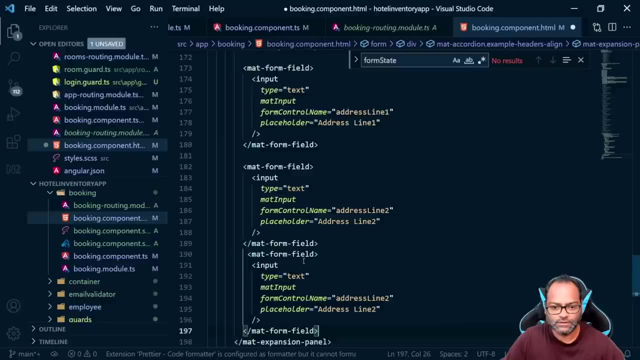 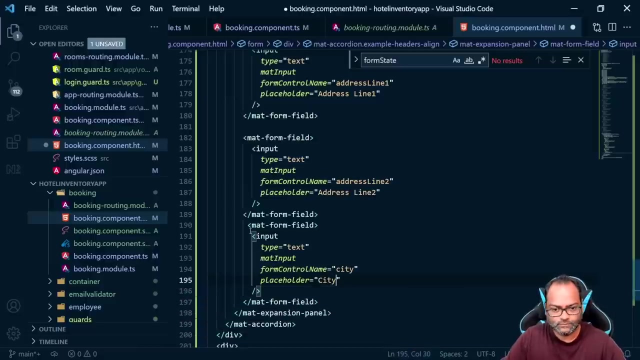 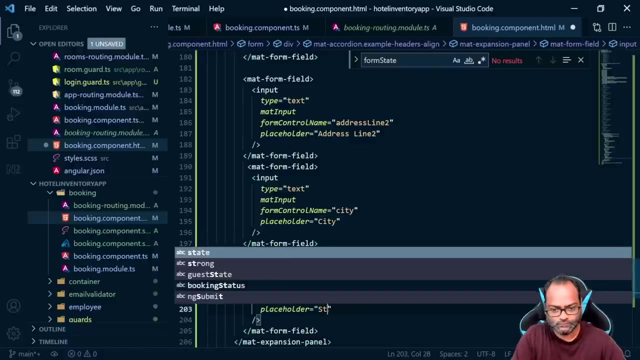 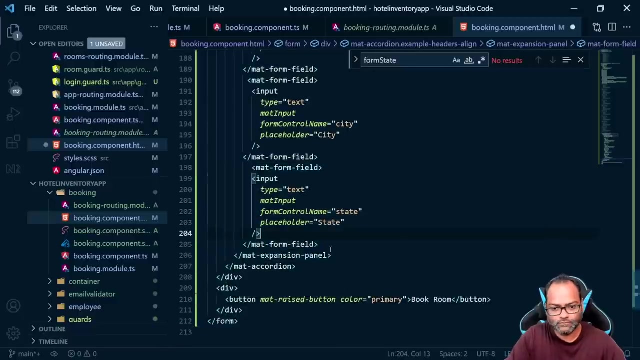 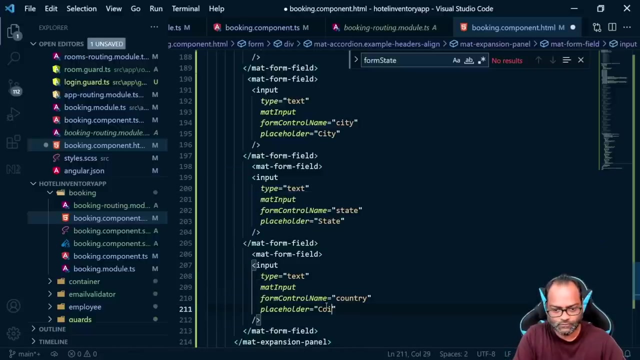 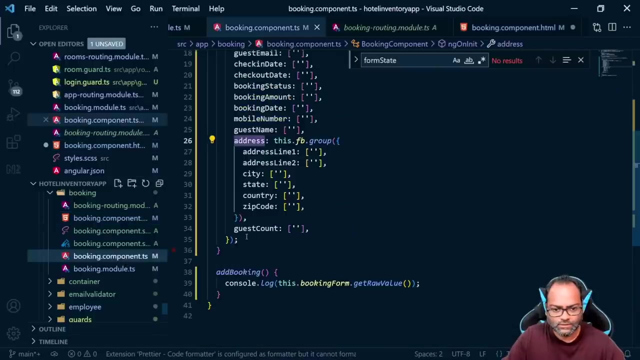 go ahead and do that. so we have address line 2. this is address line 2. and what was next? city, state, country. so let's say: this is city, city, okay, and the final is zip code. so let's see, uh, yep, zip code, or we can. 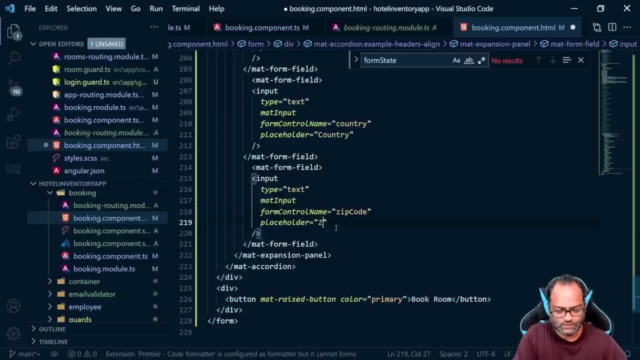 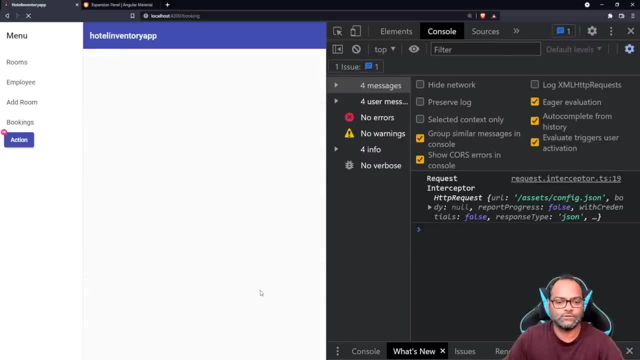 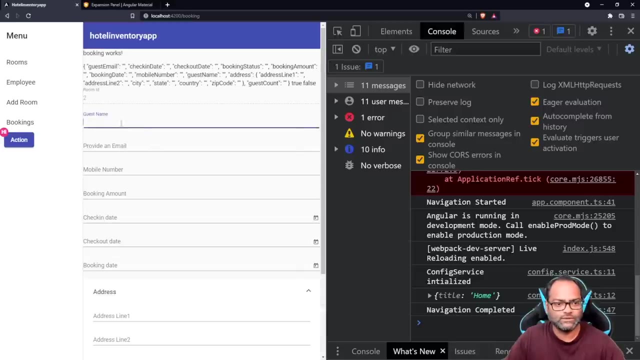 we could have just said: zip, it's absolutely fine, now we can step in. so let's see the form. so we have. uh, there's no error. it means we added all the controls successfully and now let's submit this all together. so i'll say, okay, this is this. 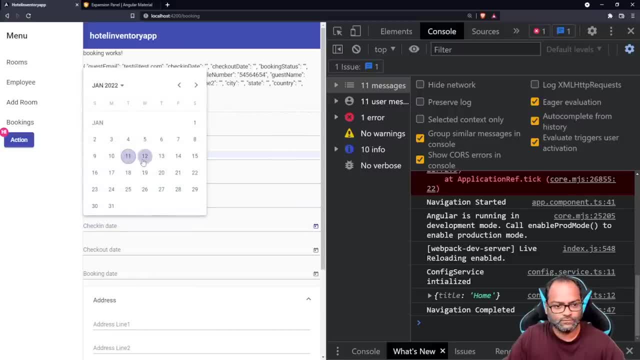 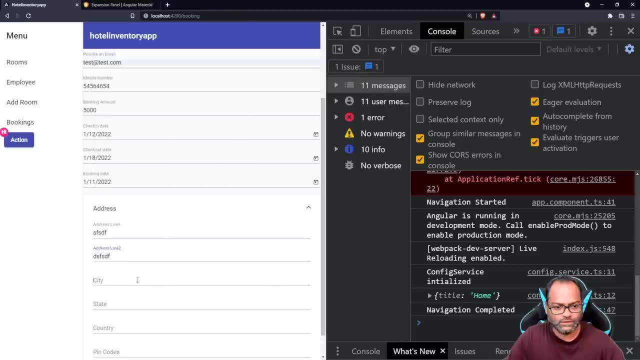 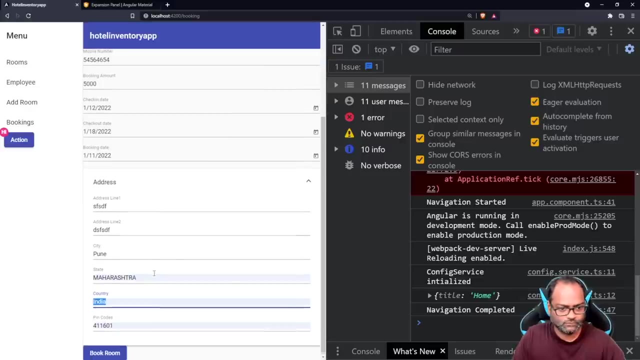 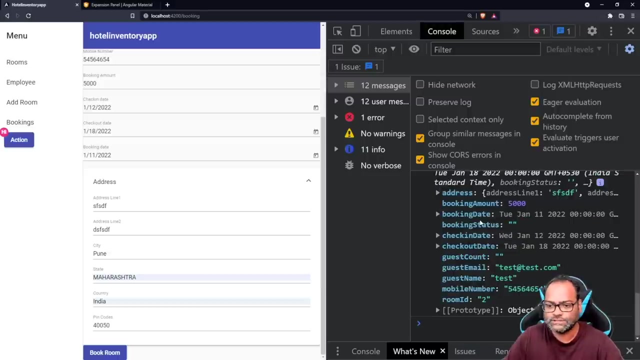 booking the mold check in date, check out date date and just find one. i just can't do. city, uh, state one right and let's click on book room. and now you have all this data available. let's see the address one right so you can see the address line one two: city, pin code. everything is available. 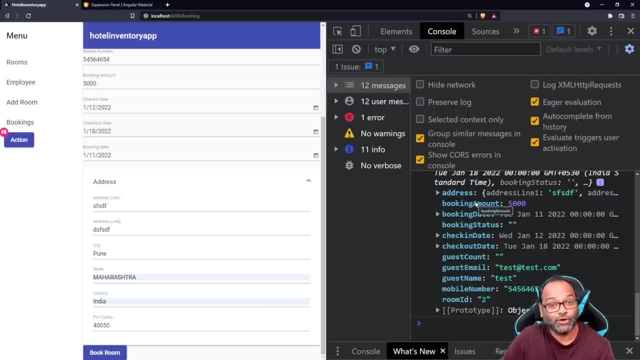 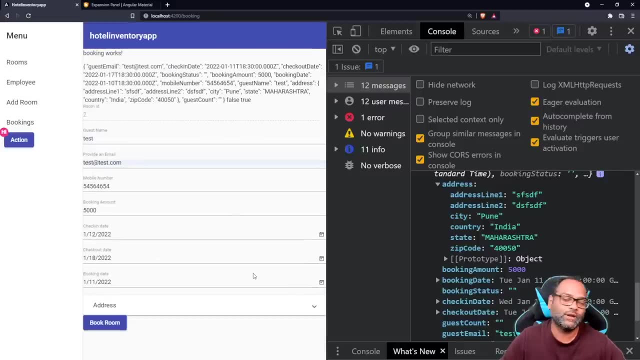 inside a net properly, uh, formatted address property, right, so you don't have to do anything. so, yep, this is how you can add nested control and this is how you can do submit. let's move on to the next, where you will see how to add controls dynamically to your form. 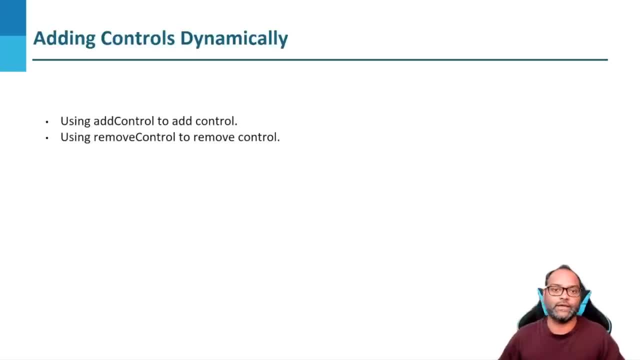 now let's go ahead and see one amazing feature which is provided by the angular forms. we will be adding and removing controls dynamically and we you will see how many uh number of lines of code we have to write to achieve this, because it's not that much, as we end up generally doing in 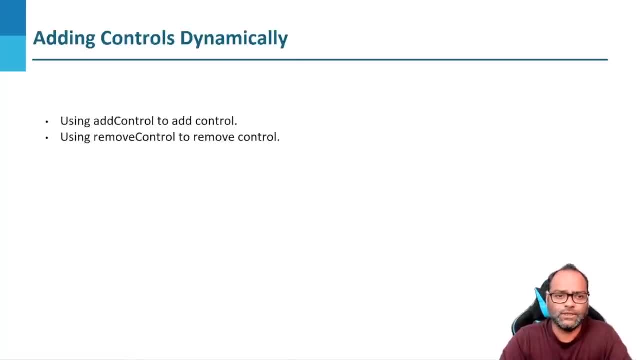 regular forms. in case you have created a dynamic form in past using jquery, you will understand the pain, or you will understand how easy it is to actually do that. i mean sorry for using the term easy, because i've been doing it from a long time. maybe it's easy for me, but yeah, you will understand at least. 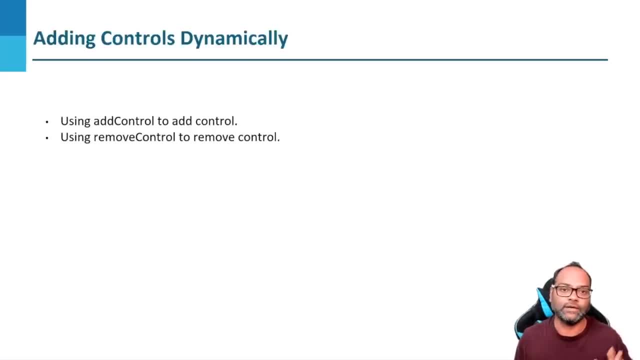 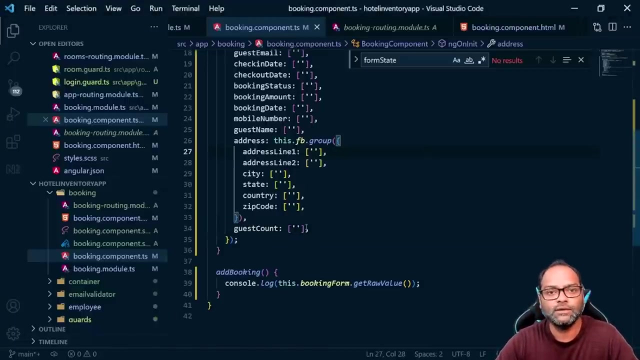 the basic difference in the api, both angular and other- uh sorry, other- framework has to offer. so let's go ahead and do that. what will be the scenario, what we are going to do here? so we will add a functionality where now, while booking, of course, it's possible, right, you can. 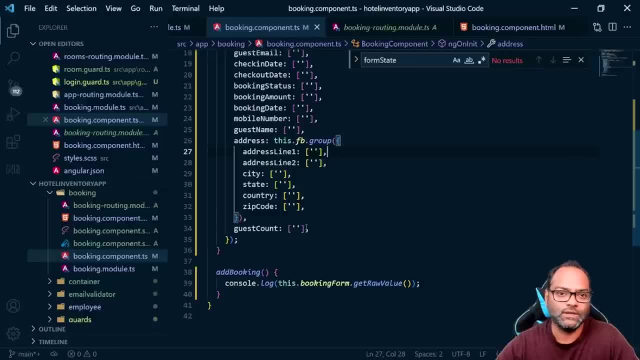 have a number of guests. you can have more. i mean three, four, whatever number of guests you want to. so we will provide a functionality where you can just click on a button which says add guest and it will add more controls as you go right. so here, rather than guest count, i'll say this will be guests. 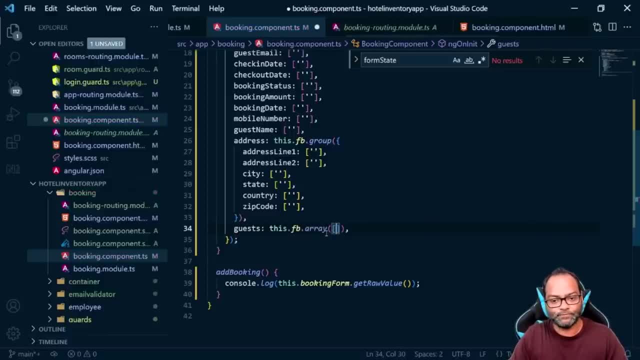 which will be this dot, fb, dot array. so we are saying now the control which we are supposed to provide will be array of controls, not the uh group. so it's it won't be a nested form, but it will be a nested form or array of a form. so here, uh, we can do something like this, so you can pass. 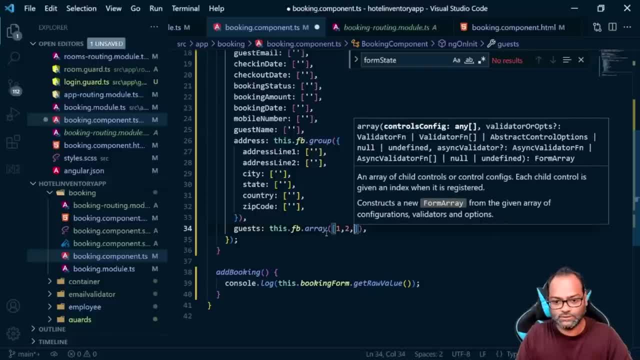 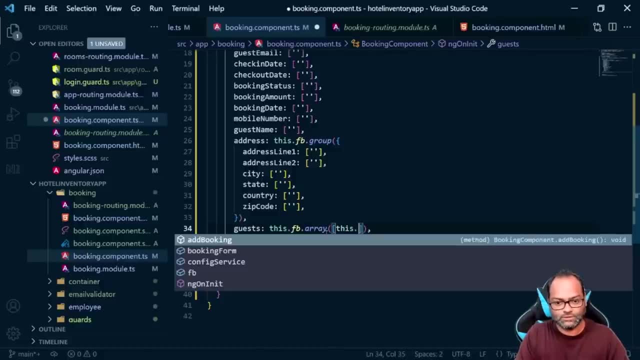 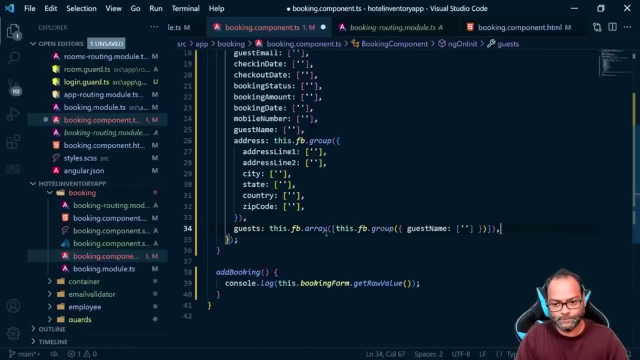 like one, two, three, something like this, right, so you can pass that number of values here. or we can also pass this dot, fp, dot group, but not control, and here i i can say, okay, this is the guest name, so it's, let's add the controls, so we have guest name: what? what we generally, uh, what? 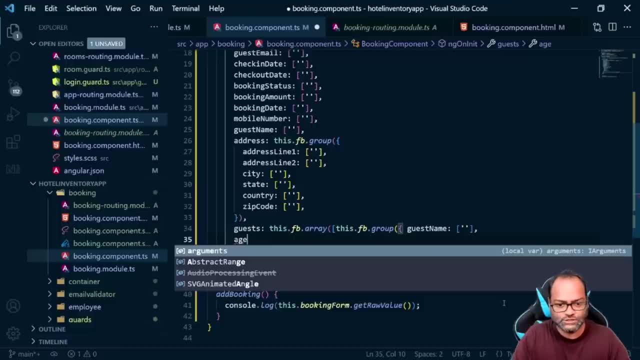 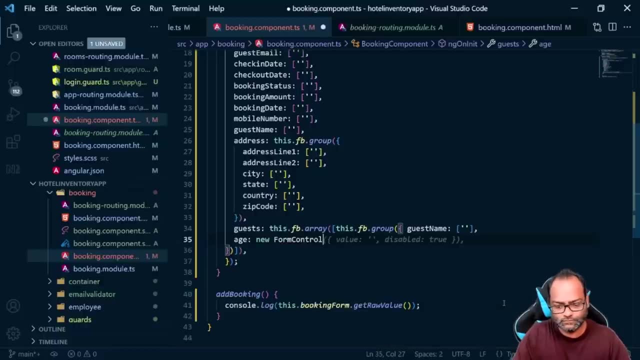 are the information we generally take. so we take name, age, right. so i'll say: this is the. this is new form control, remember. you can just use whatever way you like. you can also mix both, but follow one. i generally use this form control to get the intelligence part running. so, uh, yeah, so we get uh guest name, we get. 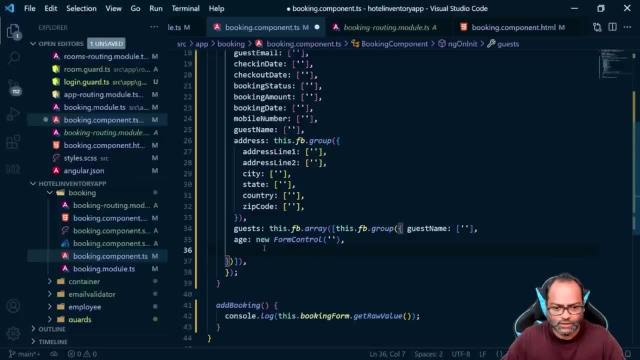 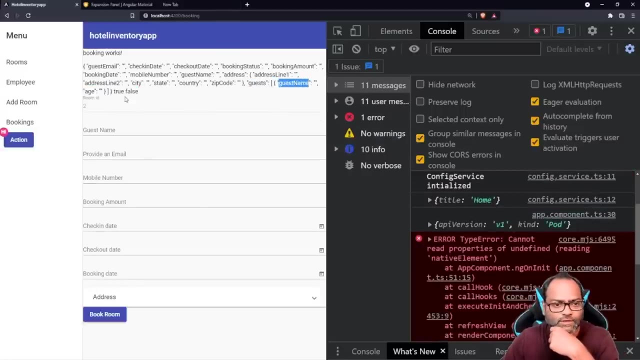 age. uh, what else? i think this is enough. let's see as of now. so let's verify this one form. so there is no error. but you can see, guest has this array right, so you have guest name and age. it means this area of a control has actually two controls available within it, and we can have an. 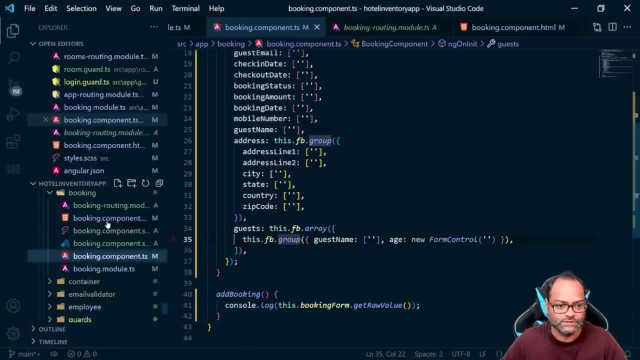 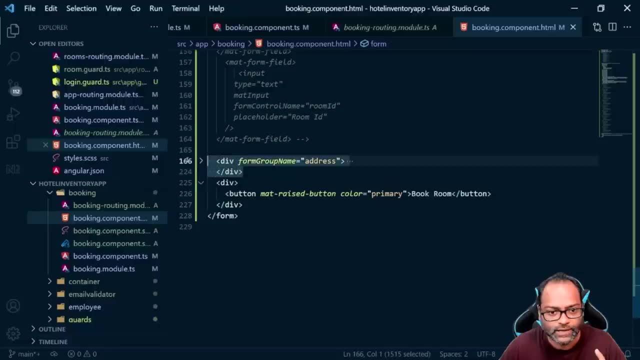 we can add n number of it. let's do one thing, let's add a button first. so remember one thing: uh, the this div is there, for instance, so i'm not going to add this new controls inside this, as as they don't belong there, they belong to. 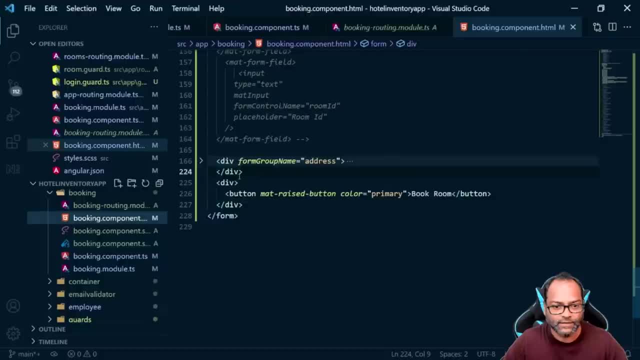 uh, this form, right, so this booking form, so i have to add it inside this form, right? so i'll just do it after this particular div and here i'll copy this button and i'll say: this is add guest and this will be type of button because, remember, if i don't give a type, 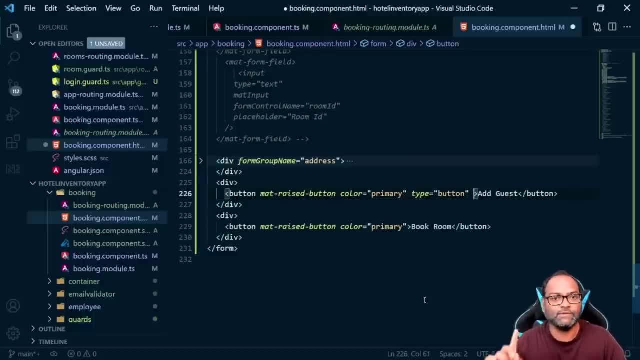 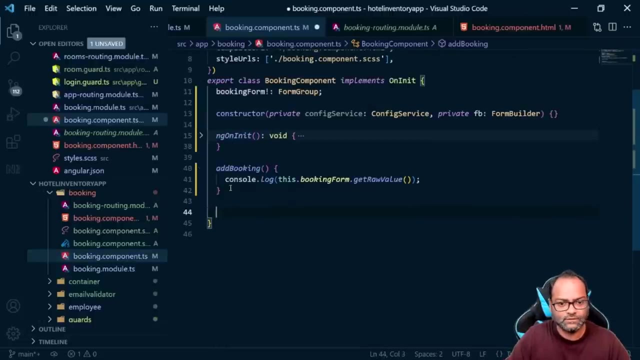 it will also submit the form, which we don't want to. we can have only one submit button within a form and on click of this button i want to add guest, so let's go ahead and see, do this. we'll write this functionality first. so let's add guest and here you can do something like this: 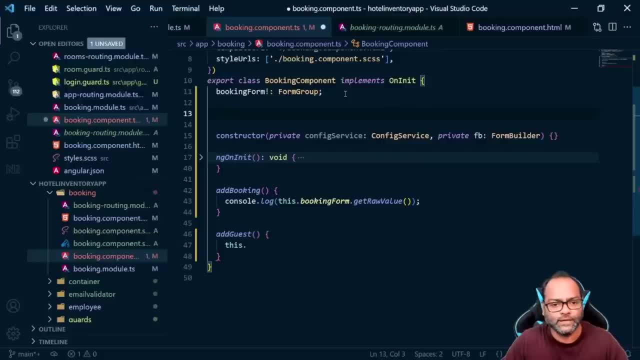 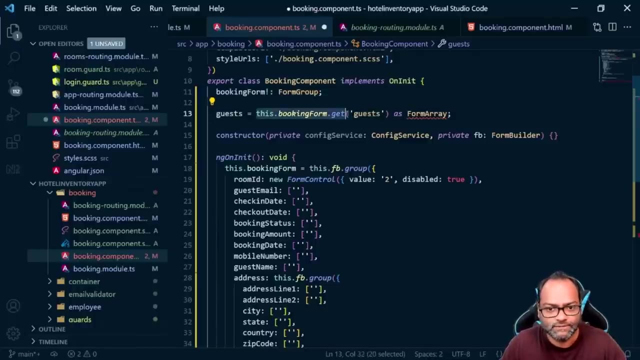 what we can do is we can create a getter property here. so let's say: this is guests is equals to this dot booking form, dot get. you can see this. you can actually access any controls by using this api, which is available inside angular reactive forms. so we can say: 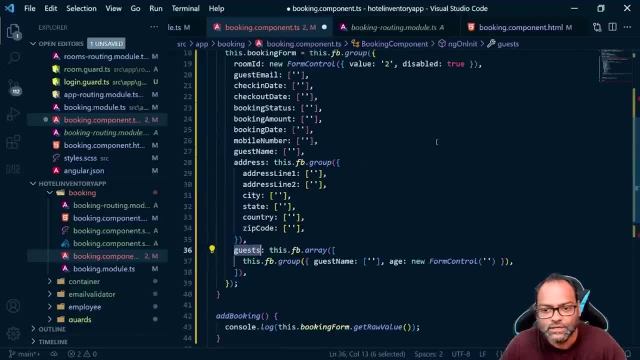 booking form, dot. get guests, which is referring to this, and we will type cast it as form array. we will tell that: okay, this is an array, this is not a control. so we will type cast it as form array. we will tell that, okay, this is an array, this is not a control. 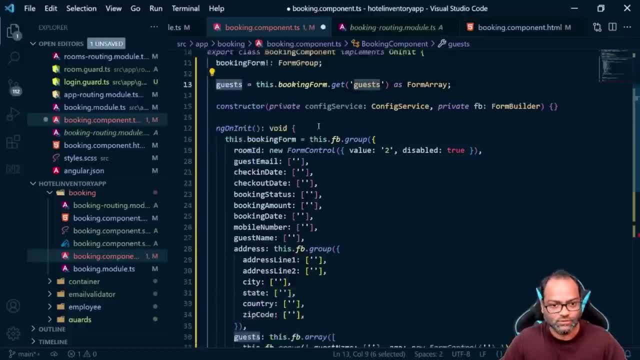 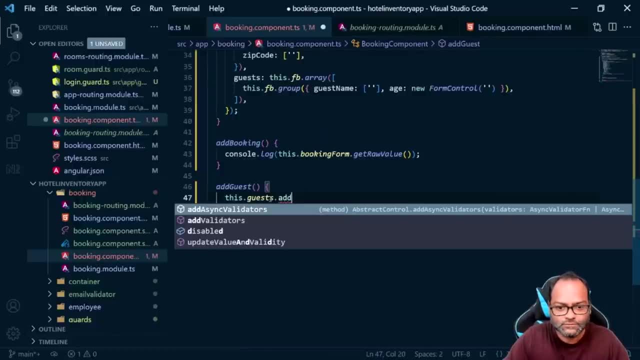 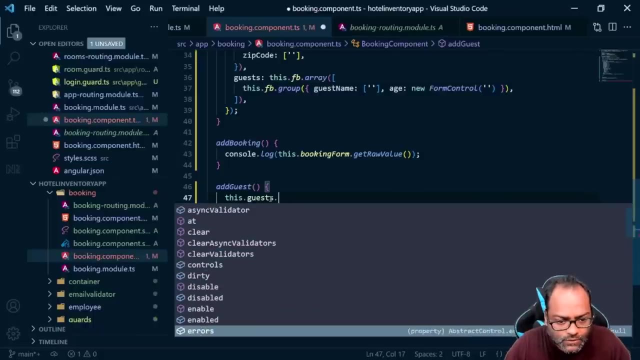 single control or this is not a nested form. so once this is done, we can do something like this, so we can say this: dot guests dot add. okay, let's see the set controls, set validators to test, test. okay, so we can say: controls dot push. okay, so we will be using this: uh, controls dot push to push a. 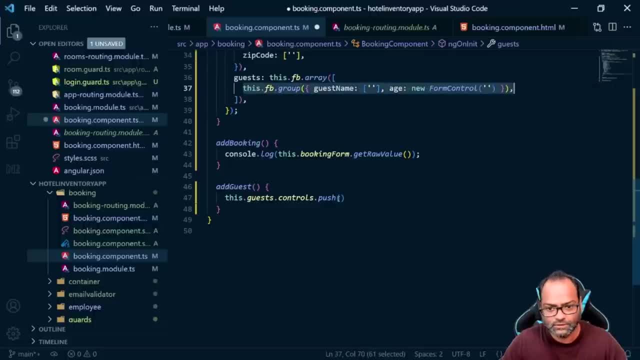 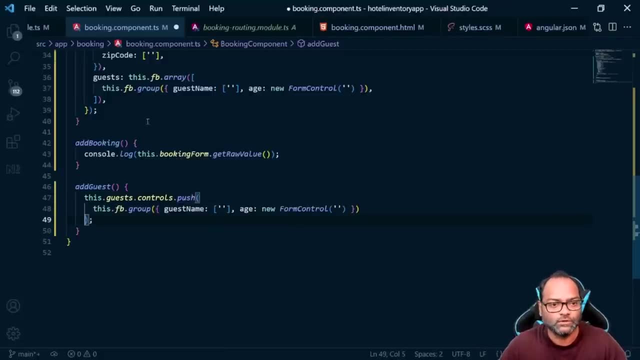 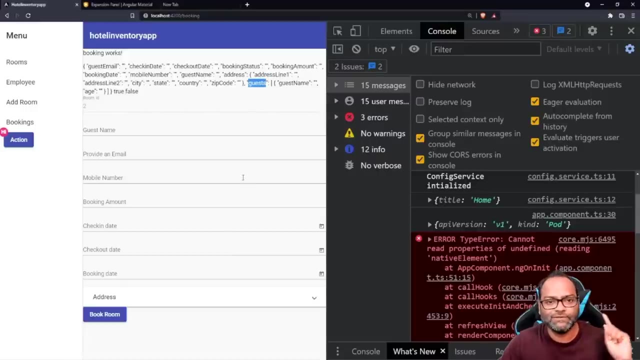 new control so we can actually do something like this. so, as this is an uh, what we can push, we can either push a control or we can push a group. so right now, it's not, of course, it's not the control which we are looking at, we are looking at a group. so let's save this and let's verify the functionality. 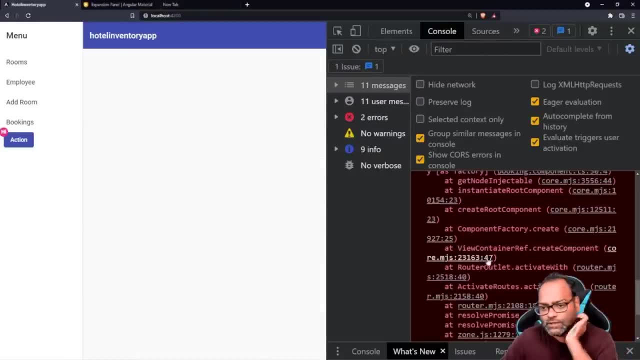 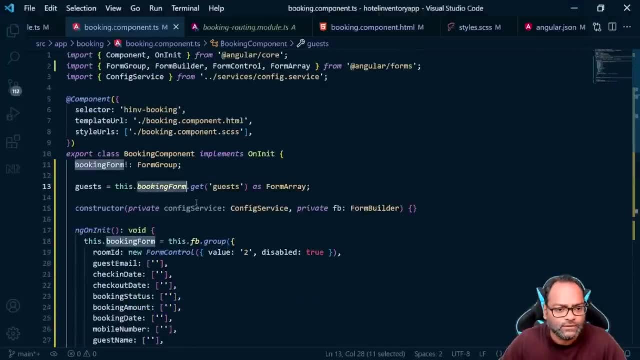 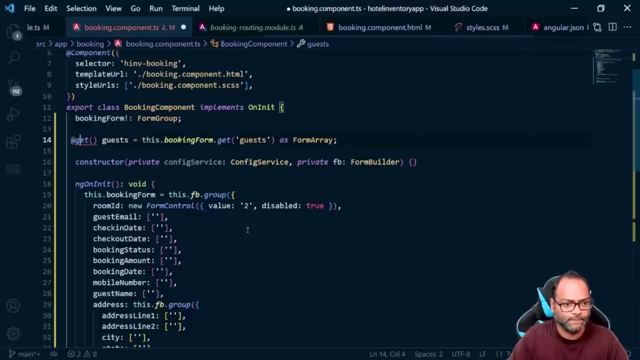 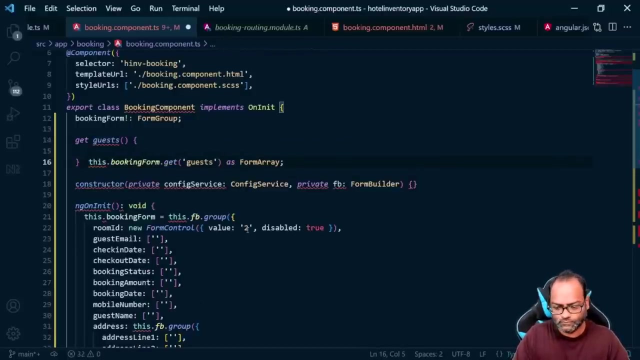 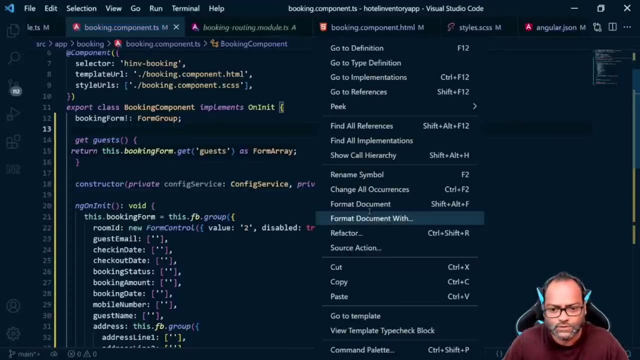 first. okay, there is some error. let's see what is this cannot read: property of undefined of get. let's see why this dot pass this what I'm doing in um and have to sayan. oh sorry, I've had written somehow the wrong syntax for getter, which. 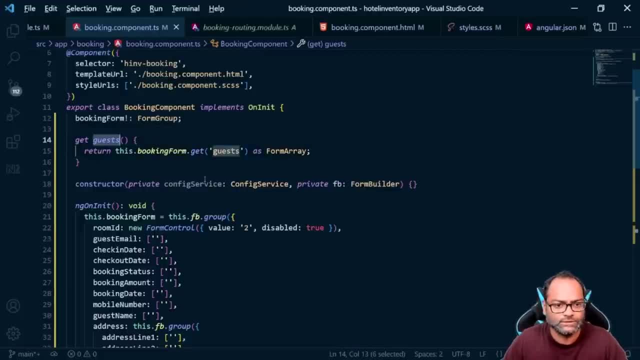 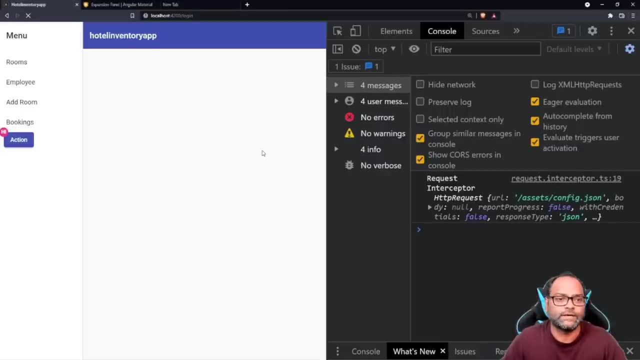 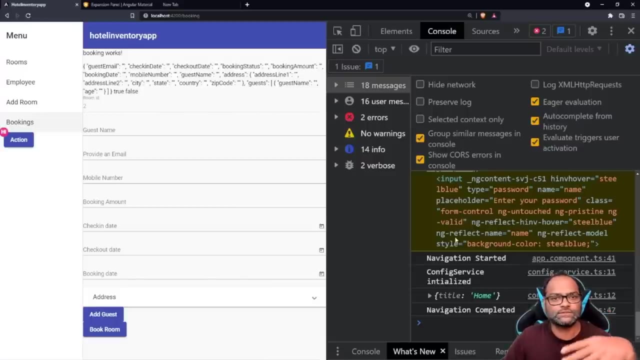 strange why I did that. so we have getter on guests. so now let's go and see get from http. no, we don't want this get from http, we want to use getter. let's go to booking and we add guest available here right. so right now, of course, we have not added this. uh, or we have not. 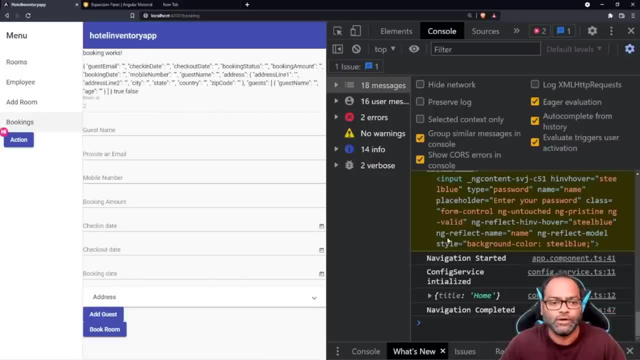 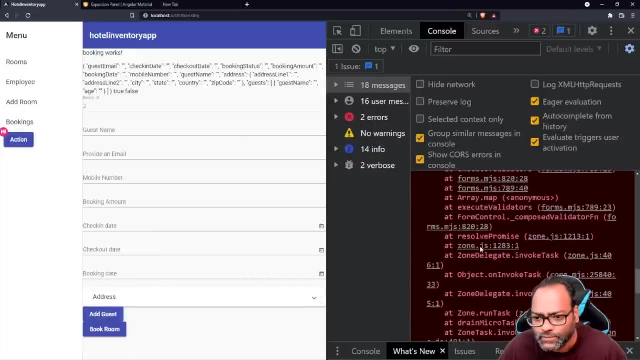 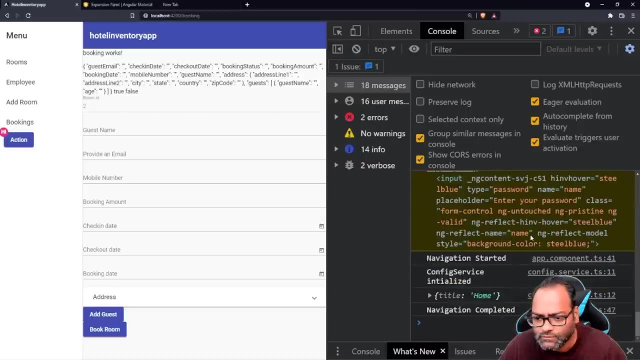 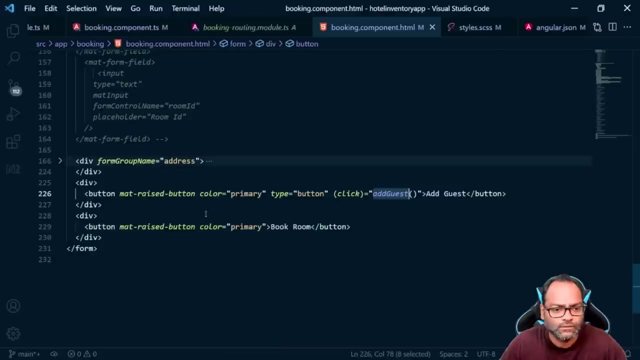 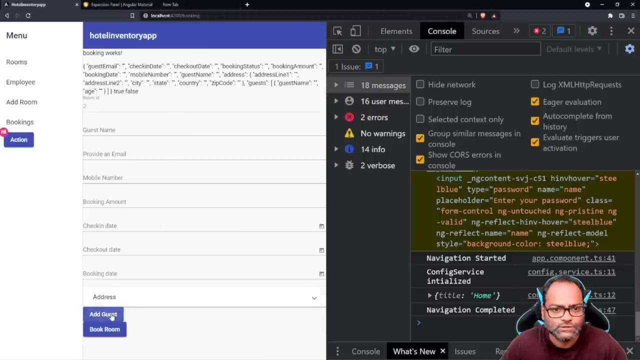 rendered this particular form group or, sorry, form array onto our view so we can click here on add guest. okay, something happened add guest but it is not doing anything. so on click, we have add guest. let's see if it is doing something strange. note guest: dot controls, dot push. 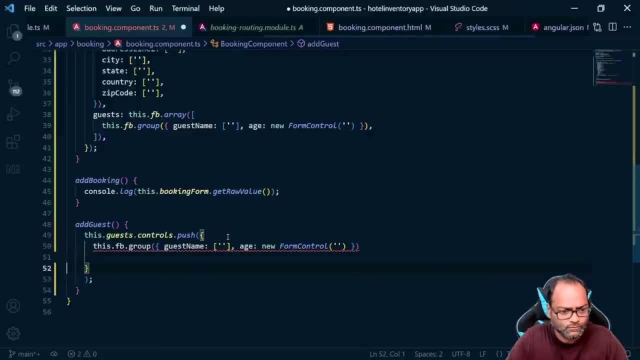 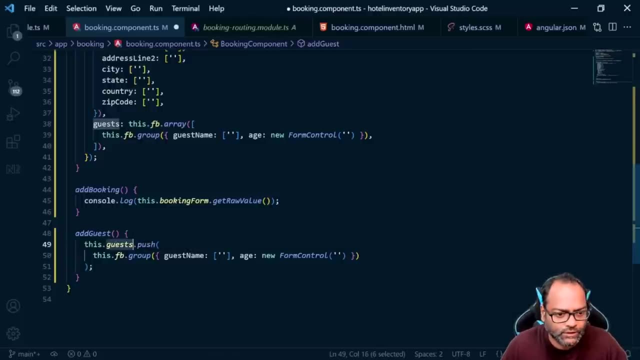 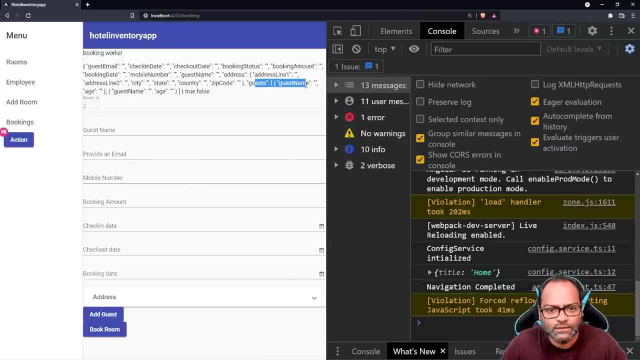 my bat. actually we need to add it to this array. so guest dot push because we don't want to go inside the controls. let's see if it works. let's click on add guest and you can see we are able to add the guests. so still, they are not rendered. so let's see if it works. 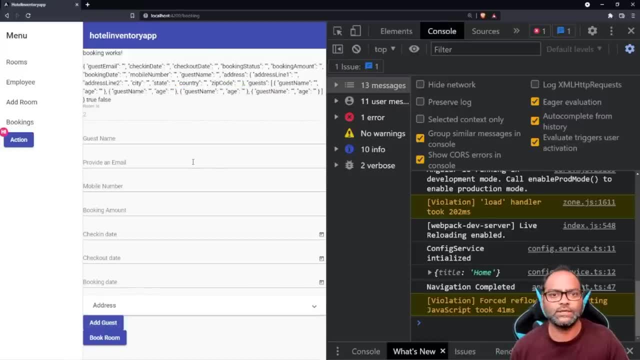 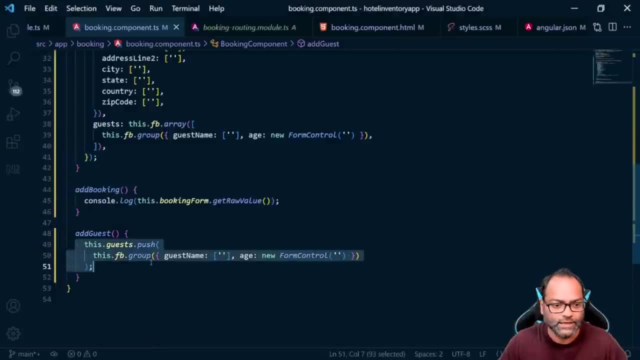 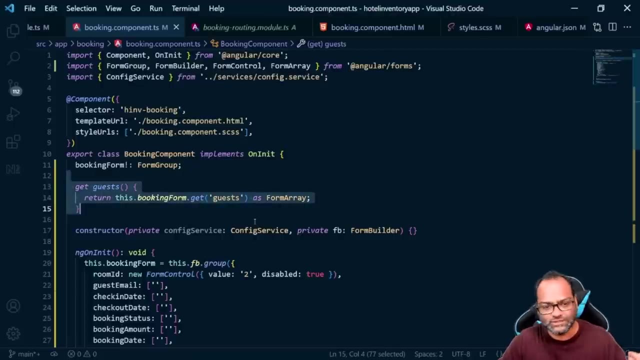 so, but yes, we are able to actually add those uh controls dynamically, right. so this is something which we, uh, we are doing, uh, we are actually adding these controls with a single line of code, remember this. so if you count this as a line, another line, so two lines of code, right, so we are doing it in. 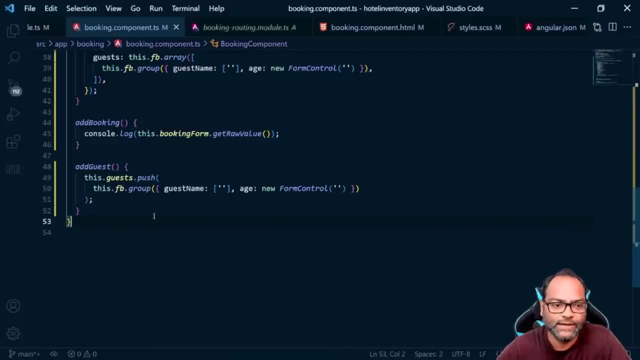 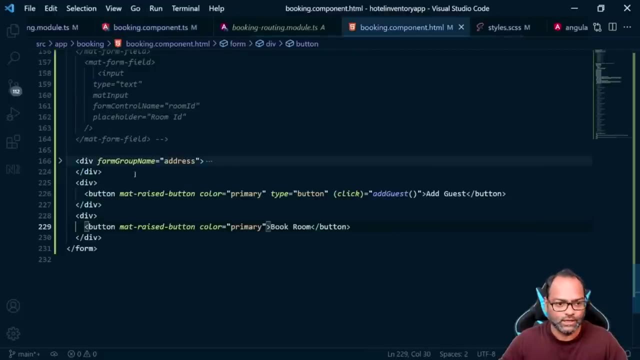 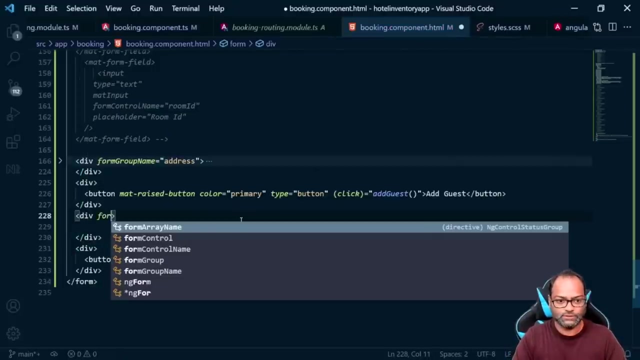 two lines of code. now let's go ahead and do the next part. let's go ahead and add it: uh, on your form, right? so we need to render this on your, on the form at the end. so, again, we'll start it with a div and here we will do something like form, array name, because we have 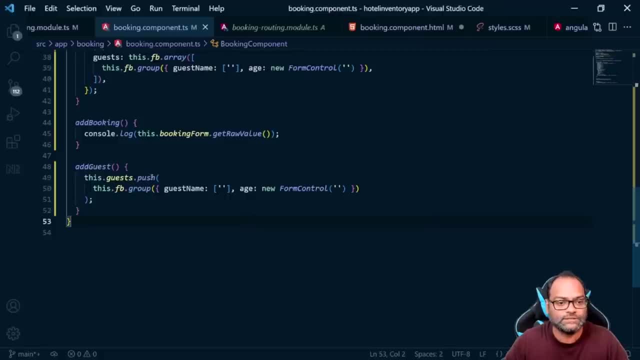 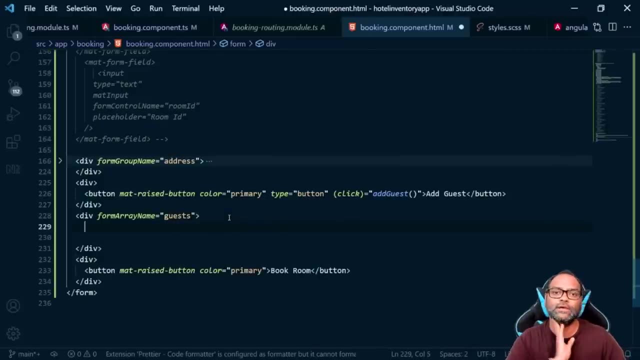 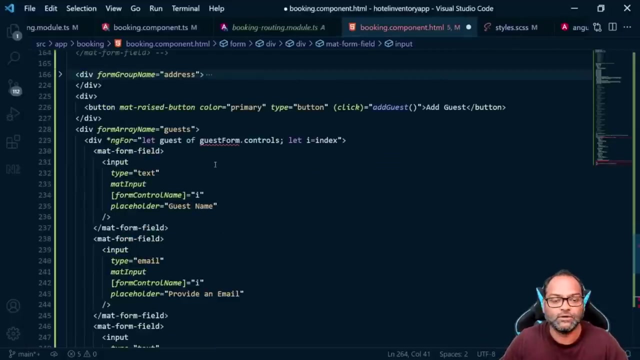 already. uh, sorry, we don't have this as a form group. we have a. it's an array. so we will say, okay, this is the guests area which we are looking at, and now here we have to go ahead and add multiple. so, uh, i'll just let me just write this code and then we'll talk about this. so here uh. 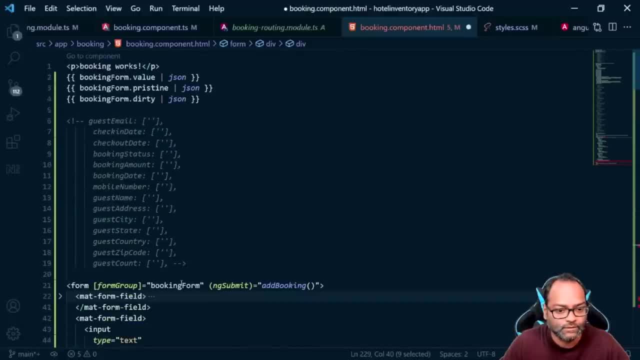 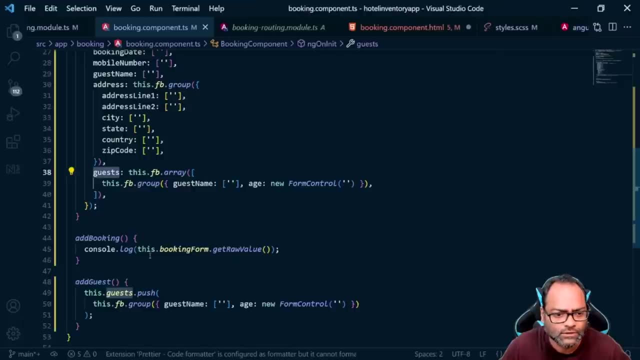 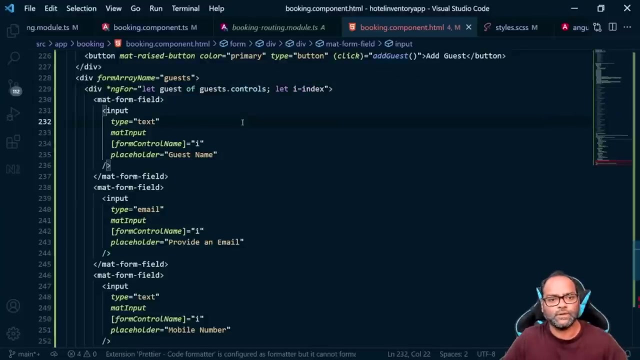 not the guest form, but we'll say booking form. uh, let's write this and then we'll talk about it, or it's not? you already have this guests dot controls. okay, and let's remove. uh, let's um, do this form control name. i will say this is. 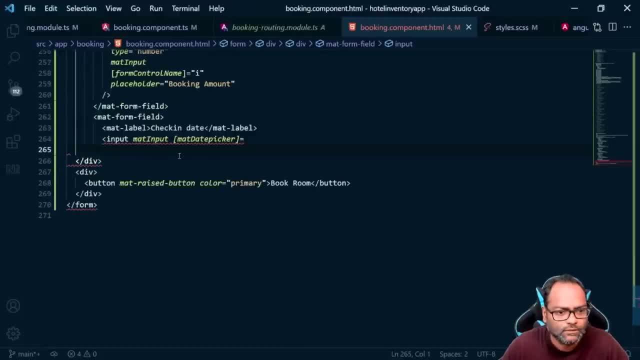 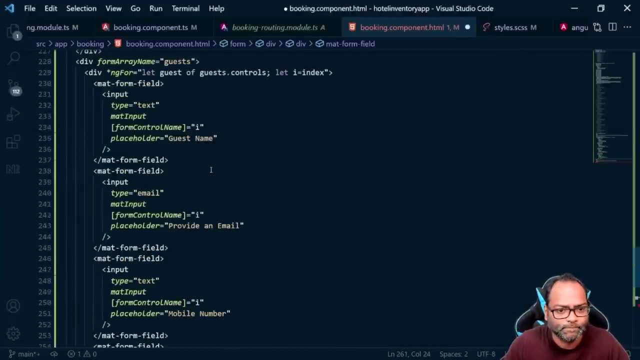 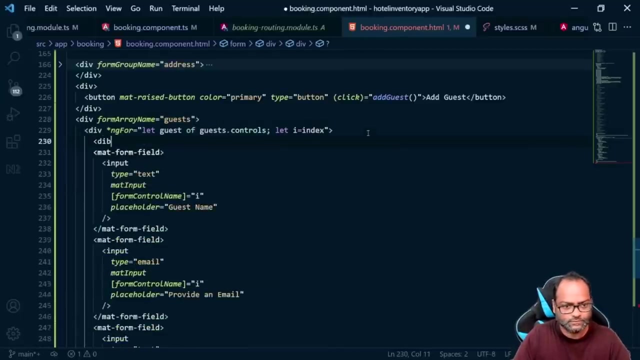 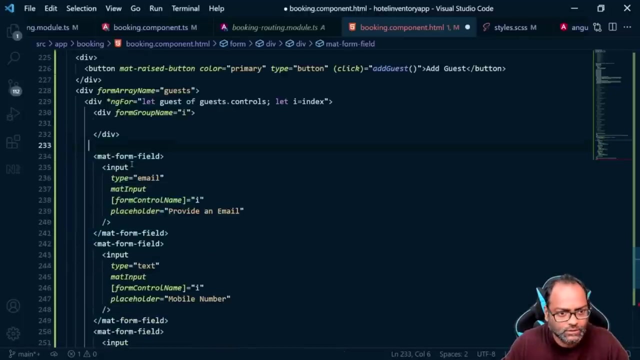 uh, this is still uh, and let's remove this. and here we wanted another div where we will use form uh. group name is equals to i, uh, so let me just complete this code and then we'll talk about what i have done. and control x- remove this extra controls- and let's see if we have matching divs. so this: 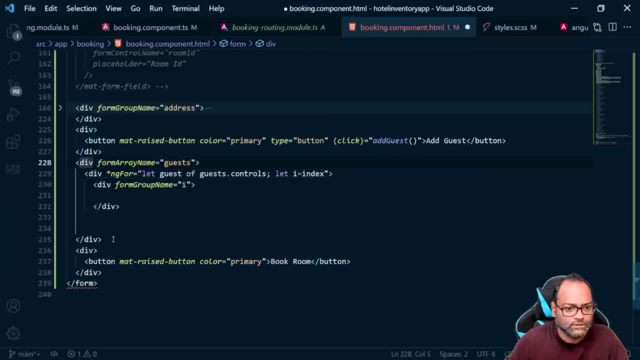 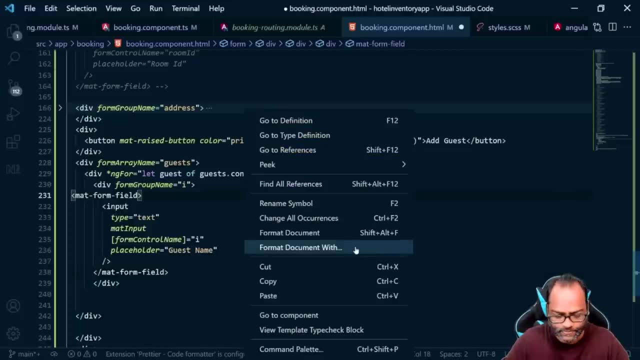 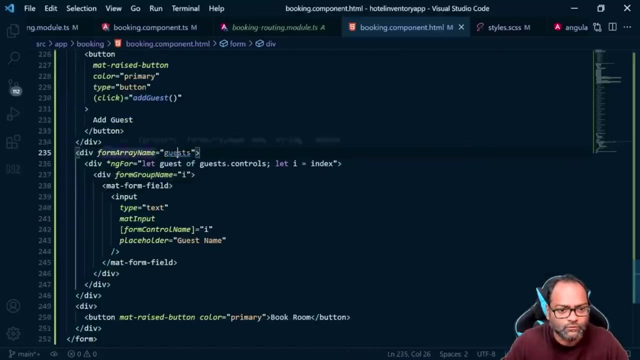 tape closes here. this tape closes here. this div does not close anywhere. so we need to close this div and okay, now it's looked fine, it looks fine, and here we will put uh form, uh. so what is the first property which we have inside guest? so it's. 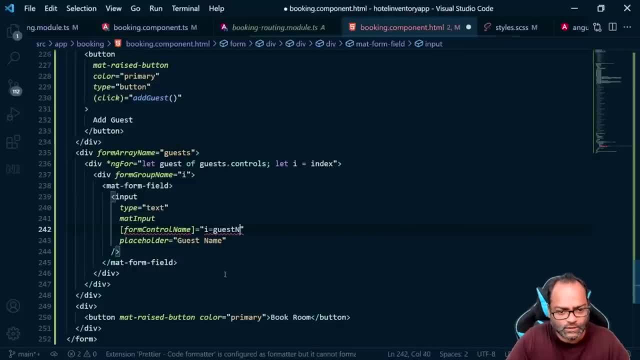 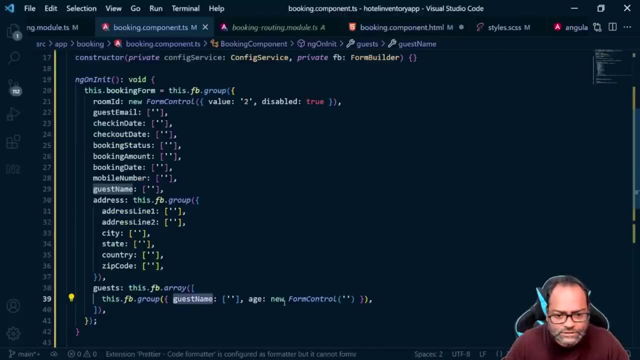 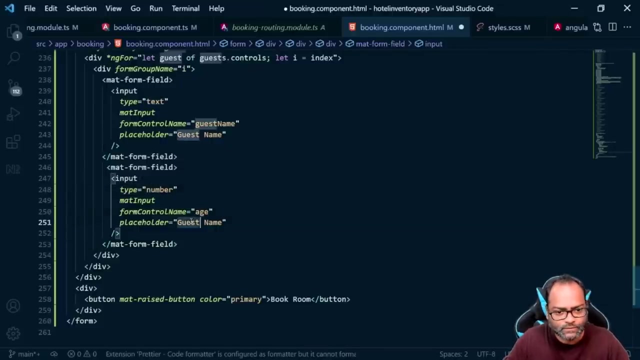 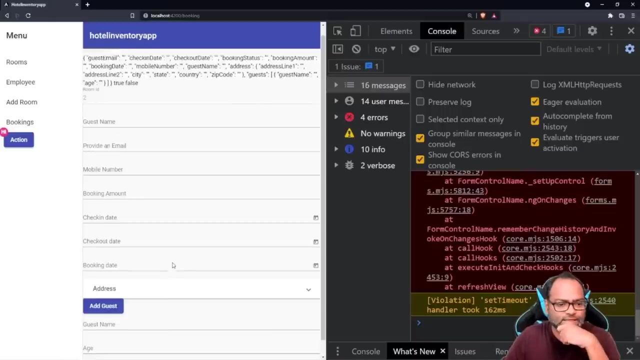 a guest name. form control name is guest name and we will use this. and similarly, we will place another form field which is of type h and so which is h and which is of type number, and let's go ahead. and so let's go ahead and see it. so you've got guest name here. let's enter something and 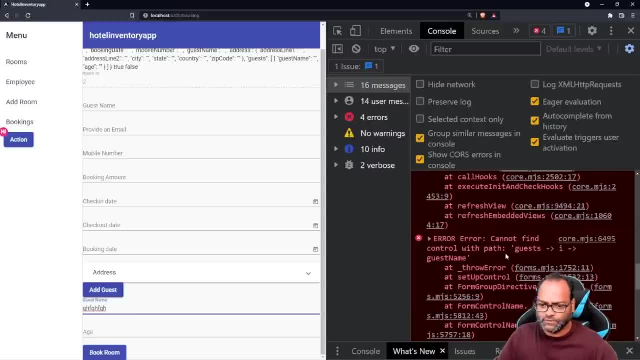 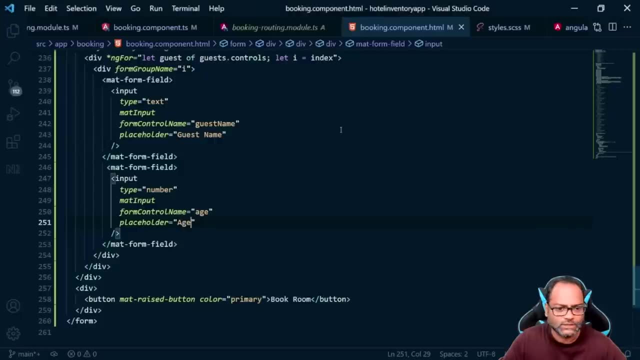 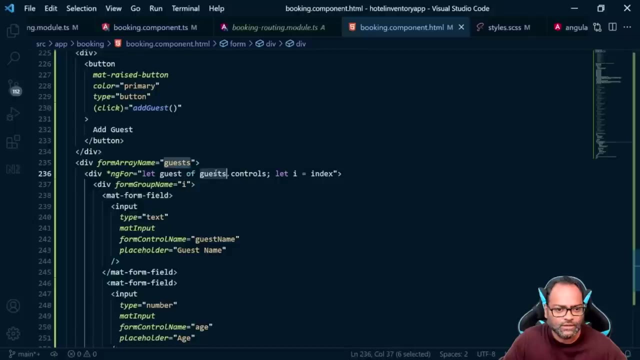 looks, looks like there is an error. so it says: okay, uh, cannot find controls with path guests i and guest name. let's go ahead and see what it is referring to. so we have a form, array, name, guess, and we are saying within each control: go ahead and look over this. 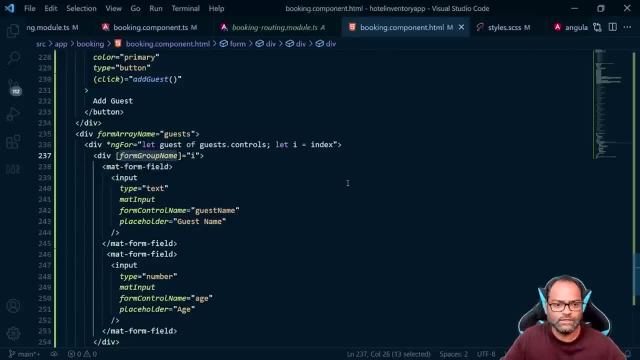 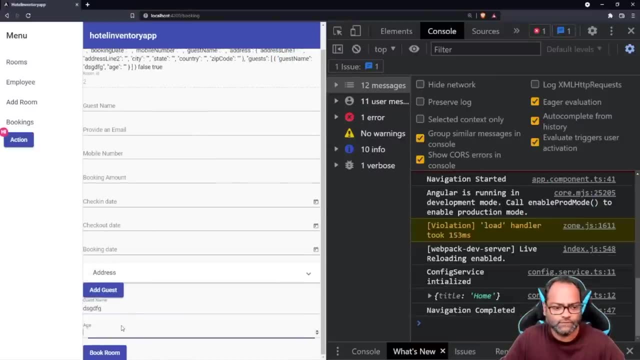 then we have form group name, and this is where the problem is over. its coordinates could have different. we have to put it in box. we'll talk about that as well. let's enter and done right. so we have our uh form working right now. let's click on add guest and you. 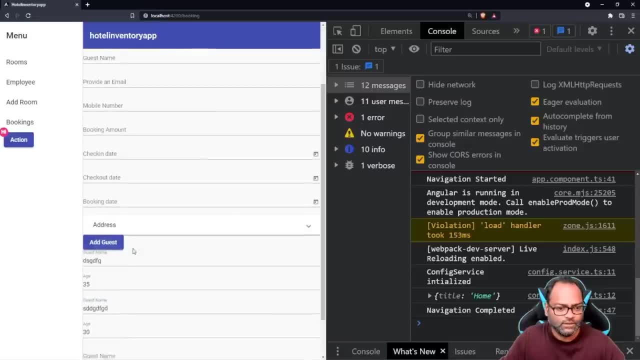 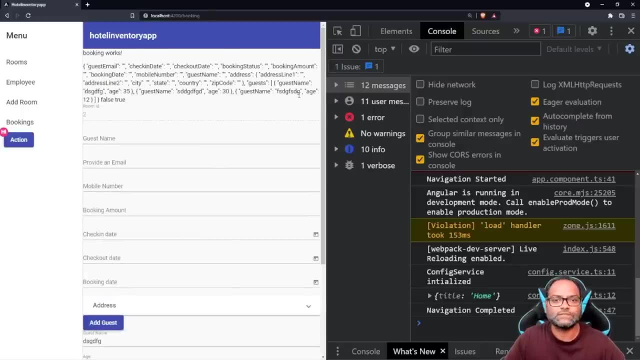 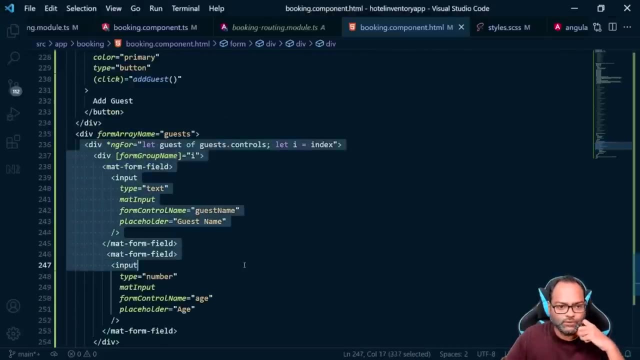 can see you have another form control, uh, which is again you can see the value available here. click on again another guest right and you can just see it is. it is in working state. so we created the form of. of course we dynamically, but we need to discuss about this. what we have done here, i mean this is really 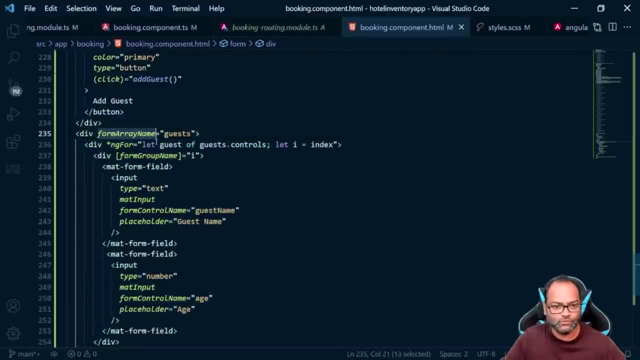 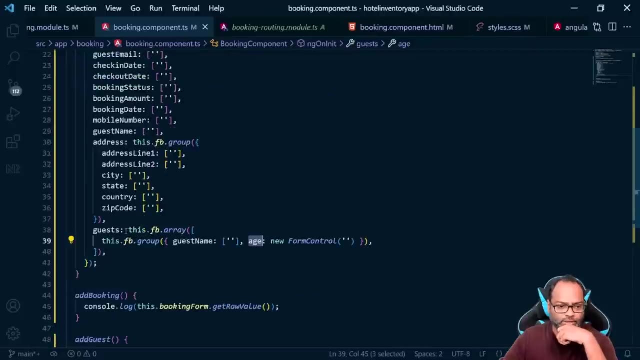 important to understand this. we know that. okay, we are referring to that. okay, this guest is in one of the form array which is available inside the form. that's why we did this. what is this logic? what is this magic? so let's go ahead and talk about it. let's go to the booking component. so 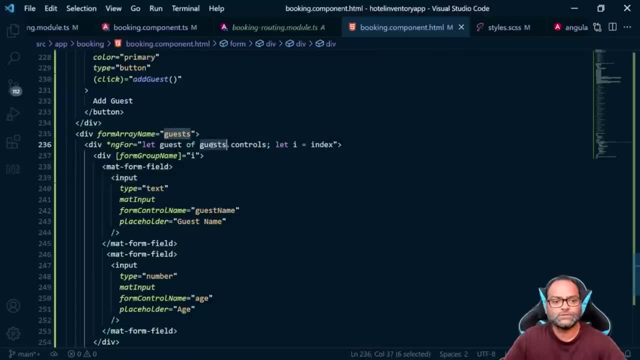 here. what we have is: uh, yeah, so what we are doing here here first. so let's try to understand this. so we are saying: now this array, this is an array, how we deal with array in angular. we have seen that. okay, in case i want to access an array of controls or, sorry, array of values, generally, we 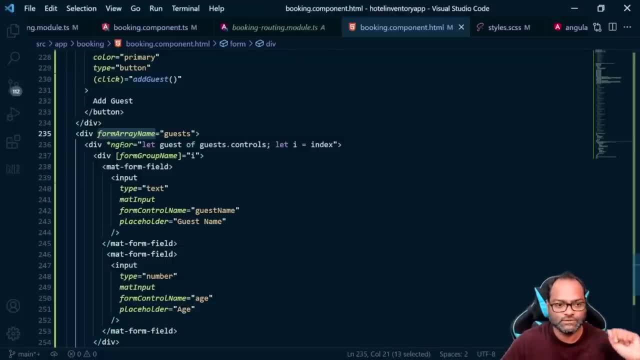 end up doing or end up writing ng for. so this is the same thing which we are doing here. so we are using ng for we are saying: go ahead and look over each and every control which is available inside this array, guest array- then this part is clear and then we are using the index value for next. 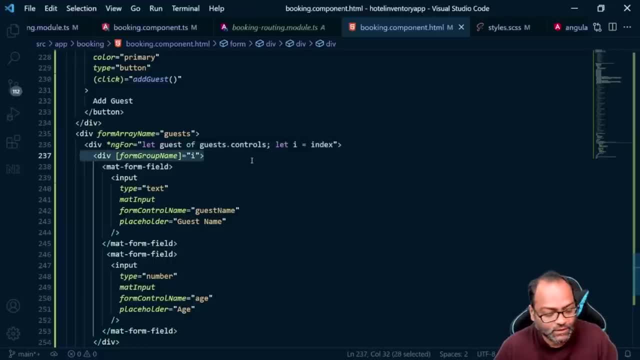 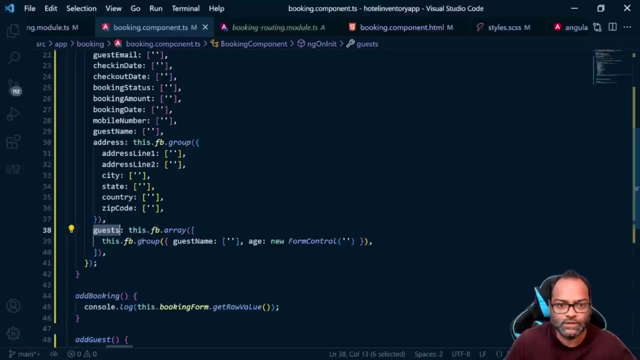 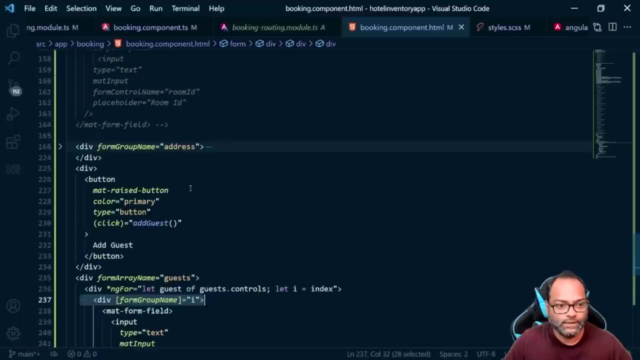 language, of course, which is available here. so form group name. so remember, let's try to understand the structure. so we have a form group, the main form group, then we have form array and then inside that form array we also have a form group. so technically i have to go ahead and use a form. 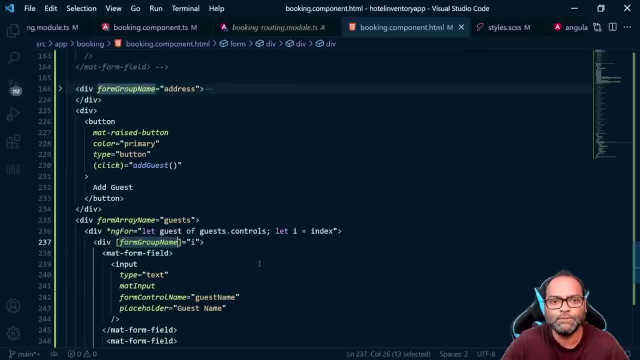 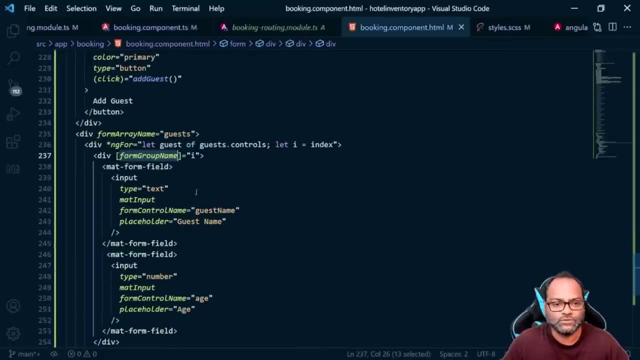 group name again here. but do we have a form group name? the answer is no, right, we don't have a form group name. we are actually just adding a form group here. it doesn't contain a name. so i have to create a form control name dynamically. so i'm saying, okay, this, i will help me to control that. 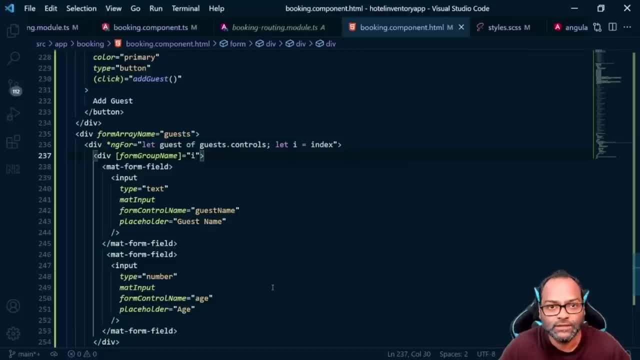 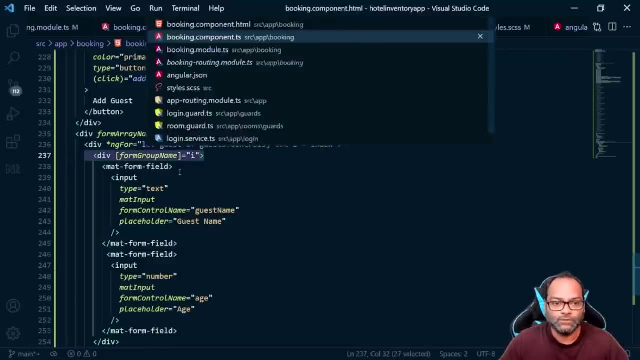 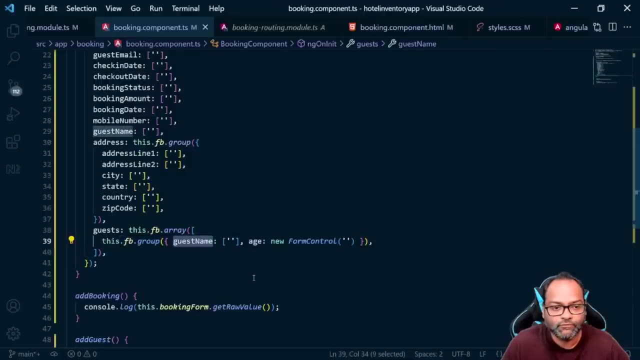 form group name dynamically, because form group name should be unique, so it starts from 0, 1, 2. so that's how it this line will help. now, once we know that, okay, this is form group name, each row will have its own unique name. the next thing which is pending is your controls. then we are just placing. 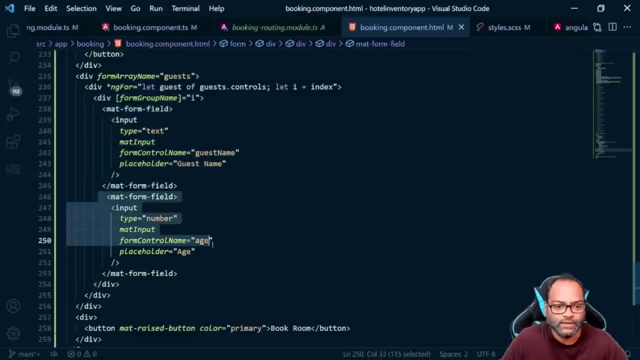 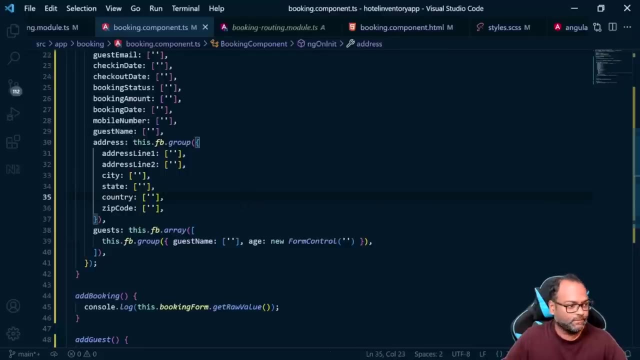 these controls inside this particular form field. and that's it, we are done. so this is what this code is. so, similarly, in case you want to add it, in your case, of course you have to do the same line. nothing will change. so once this is done- sorry, let's go ahead and see, we have this control. let's put it inside the same accordion. 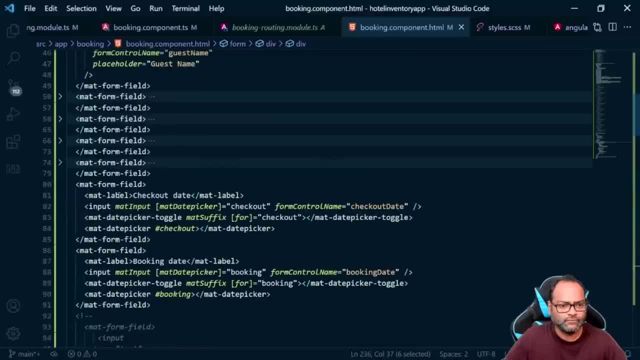 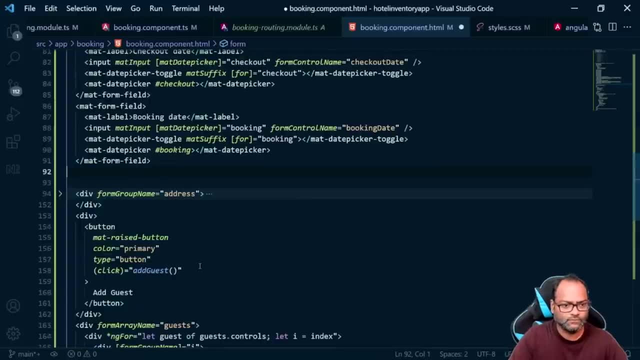 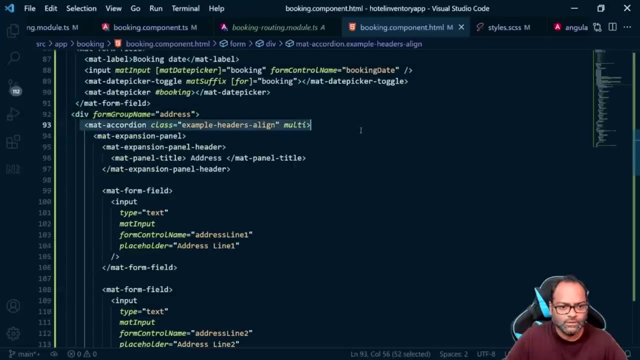 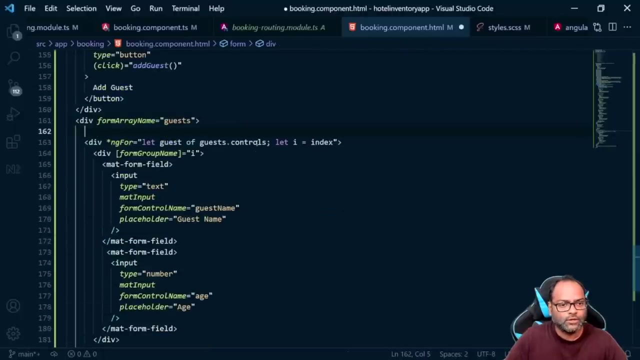 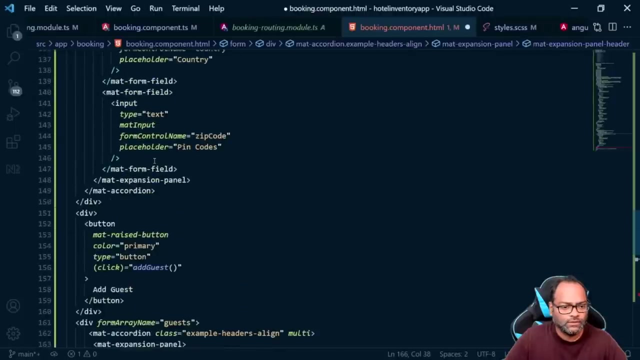 right. so let's try to do that and i'll remove this control. we don't need it. so this is our matte accordion, matte expansion panel. let's put it on top of form at a name and that's it. and then we had some closing matte expansion panel and accordion, so we'll put it here. 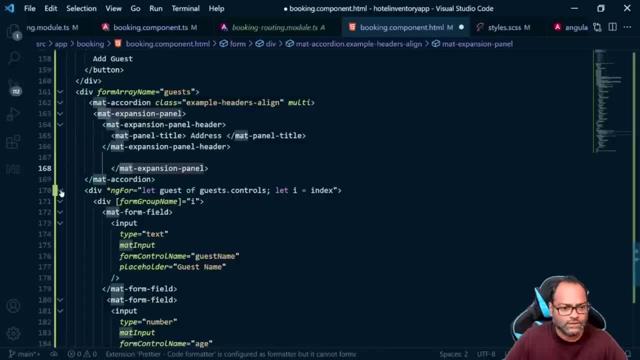 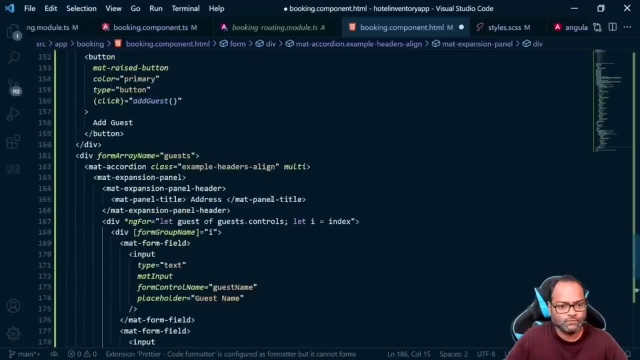 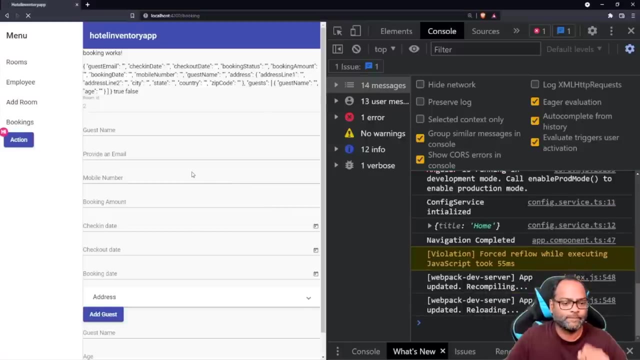 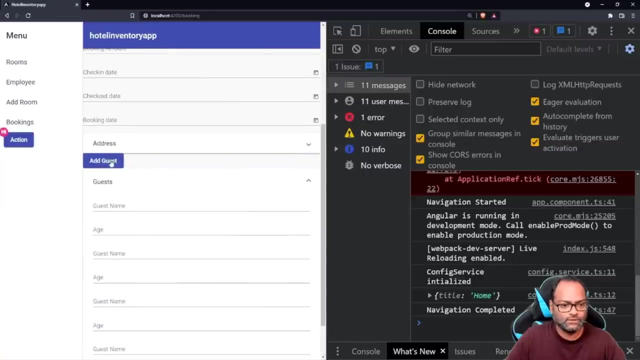 so this added, this ends here, this ends here. okay, and rather than address, we'll say guests. let's see done so. we have guests and you can add n number of guests. so within this accordion also right, so you can create multiple panels if you want to that. um, it should be guessed one, guess two, guess three, something like that. we can do that as well. 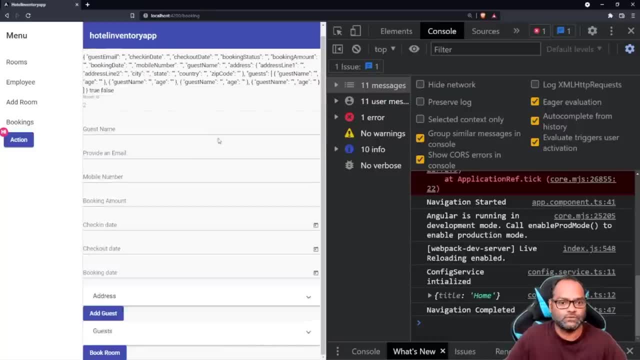 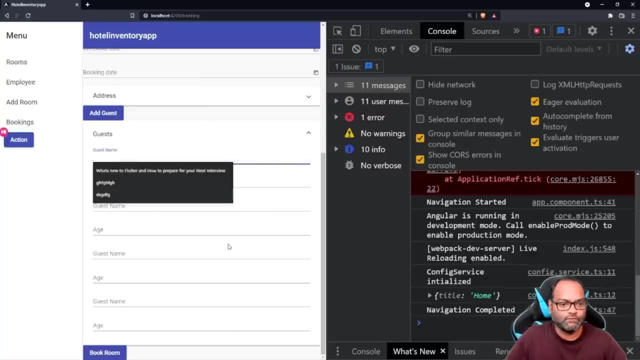 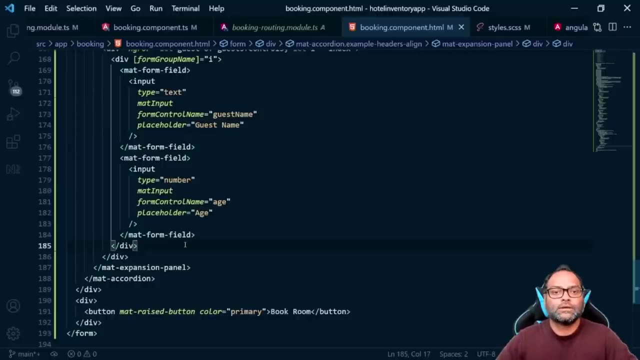 so try by your own, otherwise we will add an example. so here we will say guest. when where you click on guest, it will say guest one, guess two, guess three, something like that. so we are done, uh, adding the dynamic controls as well. we will talk about one more api, uh, which is: 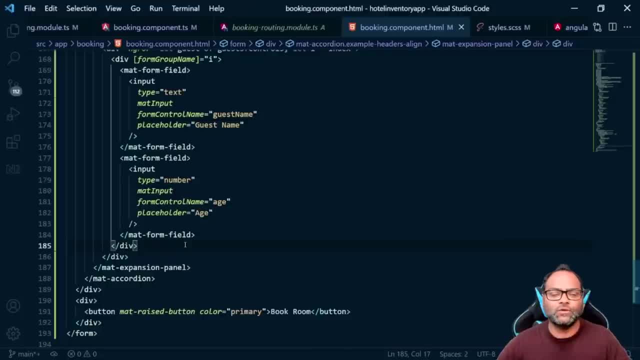 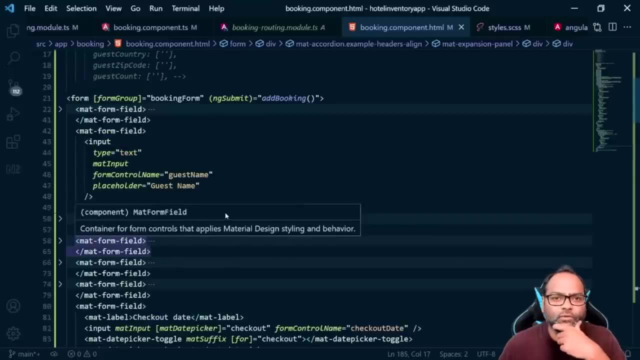 is very useful in case you want to add some extra fields. So let's take an example. Let's say there is an optional field to add a passport, Okay. so let's add a form, Let's add a button here on top. 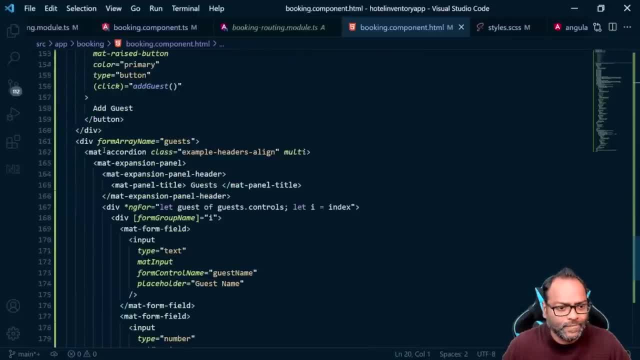 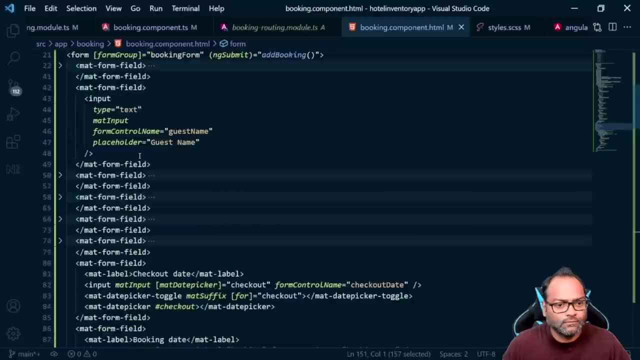 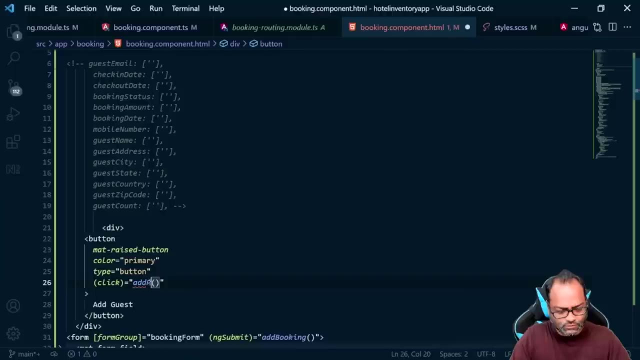 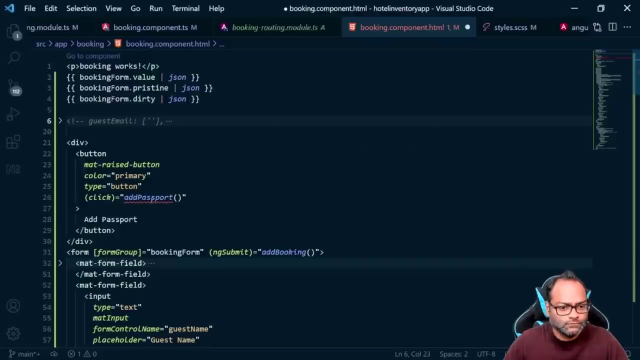 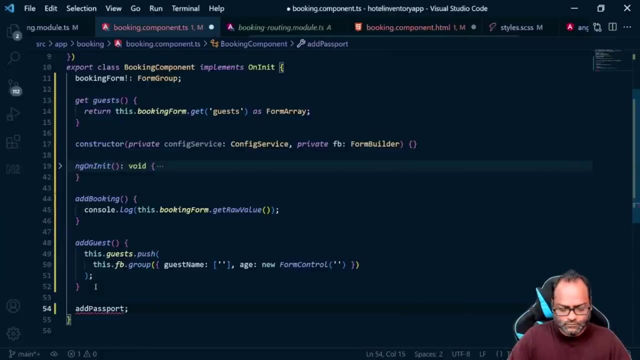 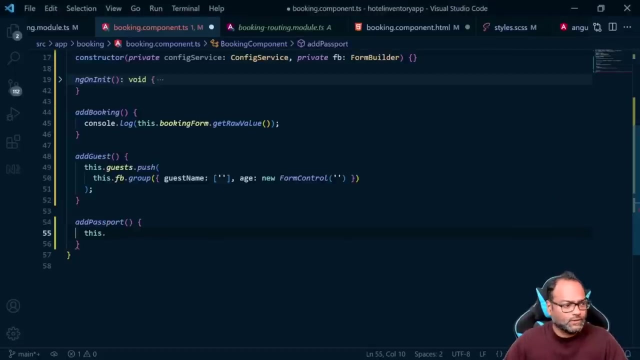 And we'll say: this is that passport, And let's implement this function. So we only want to add passport. in case we click on this button, right, It's optional. So what we can do is we can just add this dot. Let's see the API first. 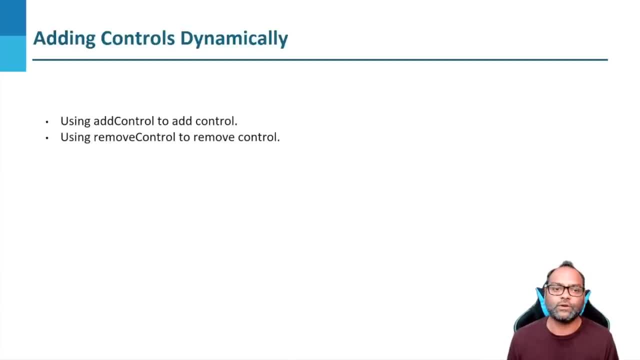 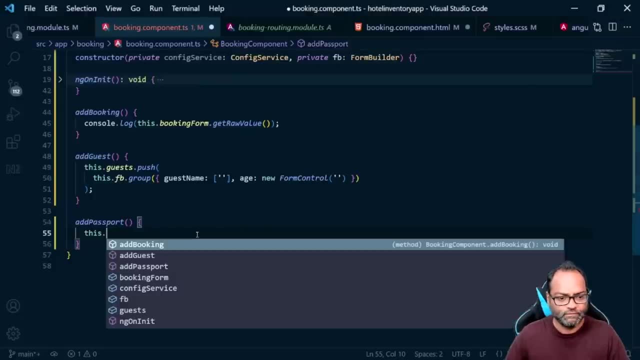 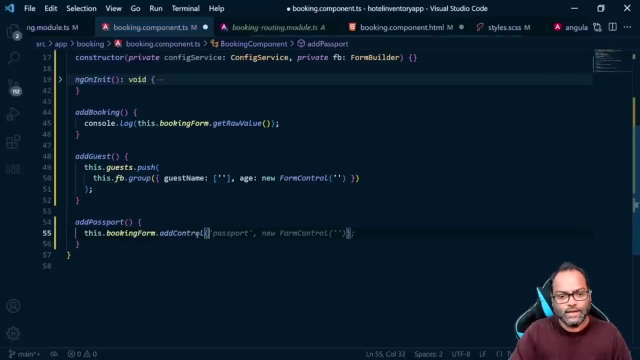 So we have something known as add control and remove control, in case you want to remove that particular control. So here we can say this: dot your form name, So this is booking form. dot. add control And as it says control, so we'll be adding one control. 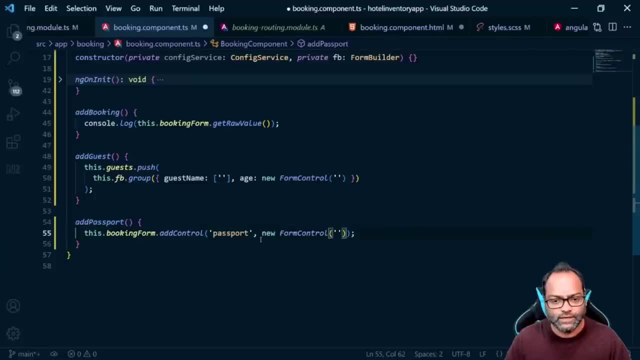 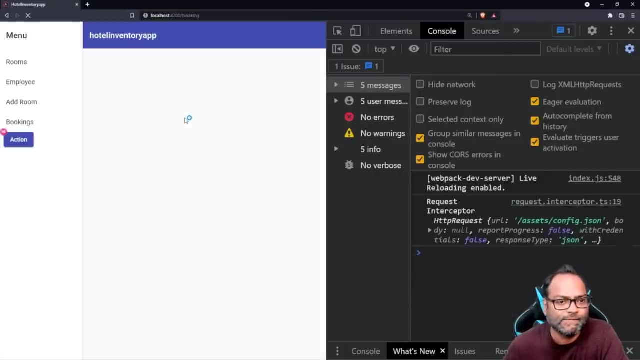 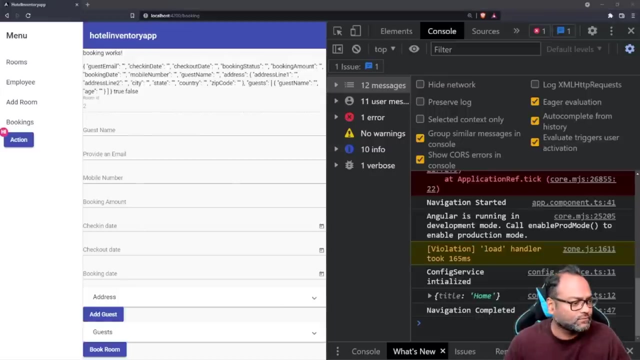 So we can say, okay, this control name is passport and we can choose to have a default value, right, So let's go ahead and see. So, of course, it's not available here right now. Let's click on the button. 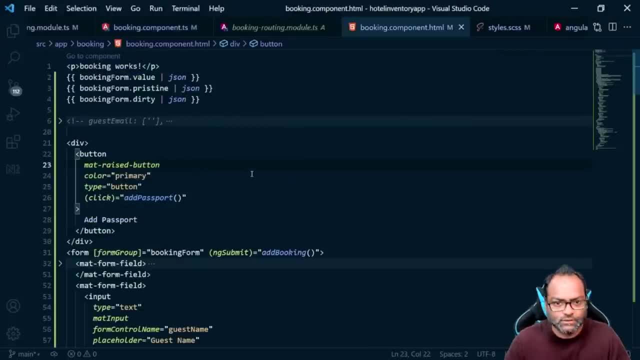 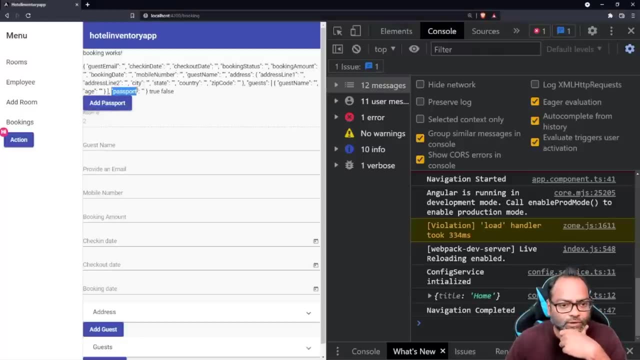 And for that we have to save this form And let's see. So we click on add passport and you can see a new form control called passport is available here. So this is just in case we need some extra information, right? So you can actually do that by using the. 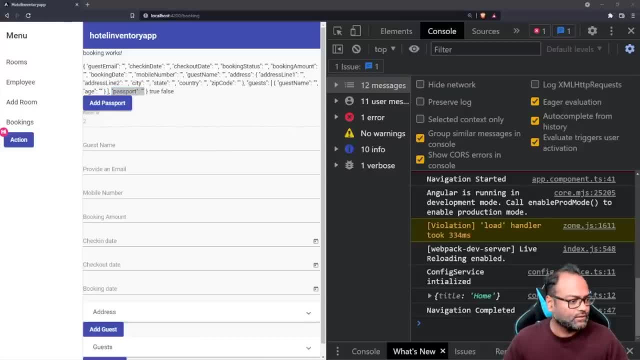 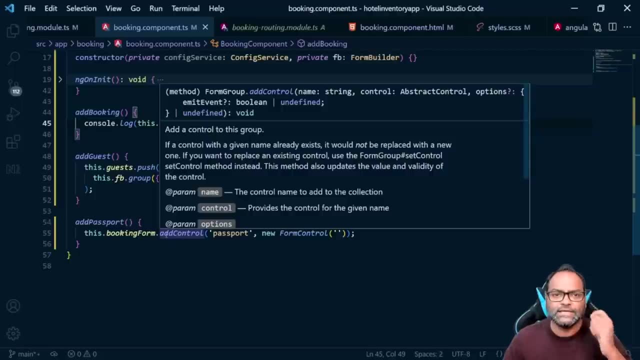 add control API, which exists. You can remove the same using the remove control, But let's let's see how to bind it, because what in case? this control does not exist, right? So here let's see how we can add it. 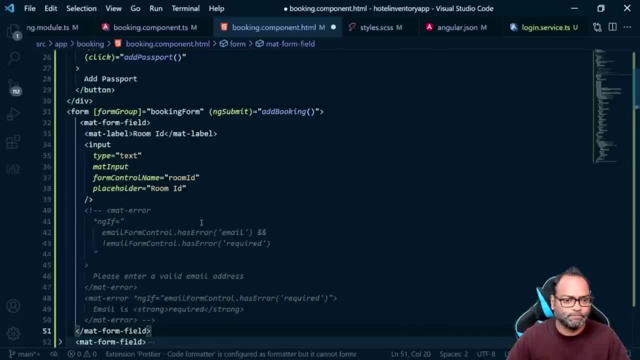 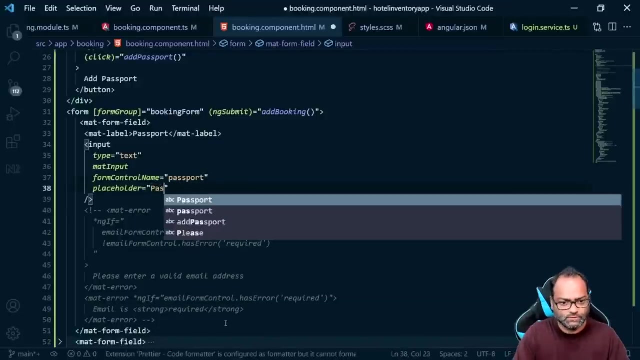 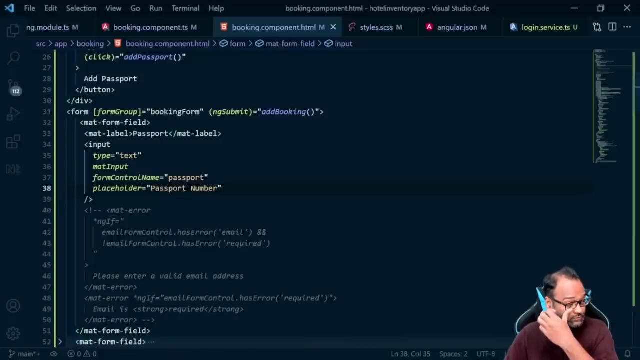 So I just add one matform field And we'll say this is passport, And we'll say this is the control name is passport And this folder name is passport number. But if I try to add this right now, let's see. 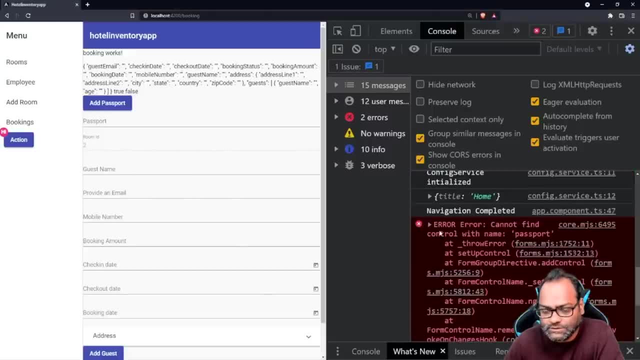 So if you try to add this right now, you will get an exception because, right currently this form control does not exist. Right So it does not exist and it will throw an exception. So if you try to add this right now, you will get an exception because, right currently, this form control does not exist. So if you try to add this right now, you will get an exception because right currently this form control does not exist. So if you try to add this right now, you will get an exception because right currently this form control does not exist. 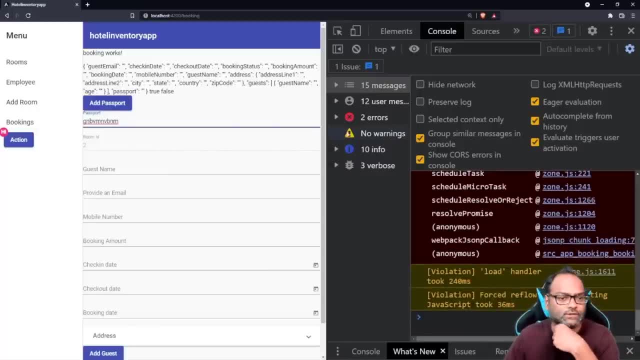 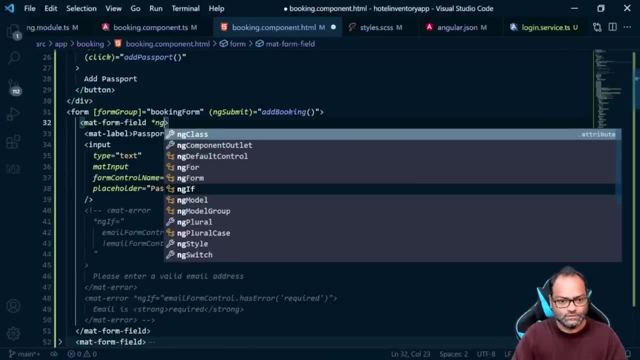 If you click on the passport and now enter, as there was already an error, it will not work. How do I handle this scenario? So we can use ngf, right, So we can say ngf. we can say, okay, this dot. 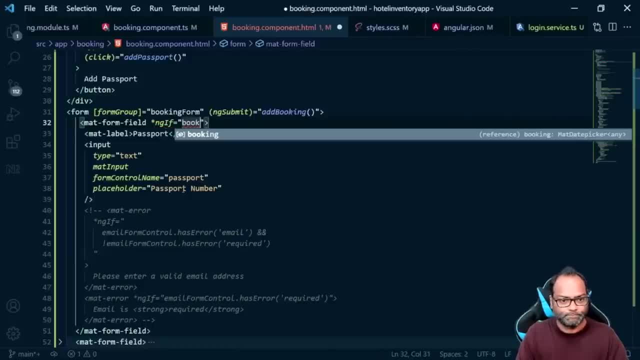 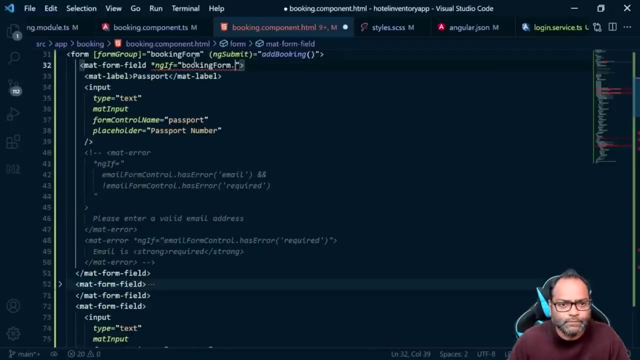 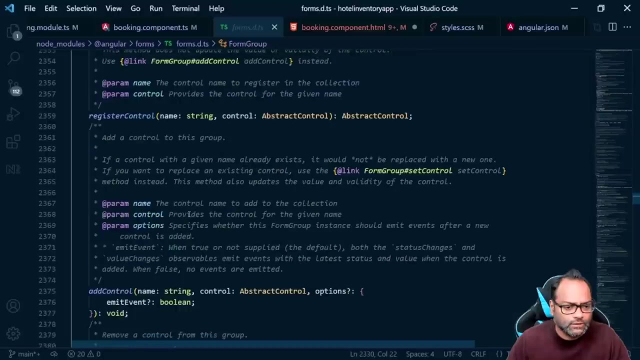 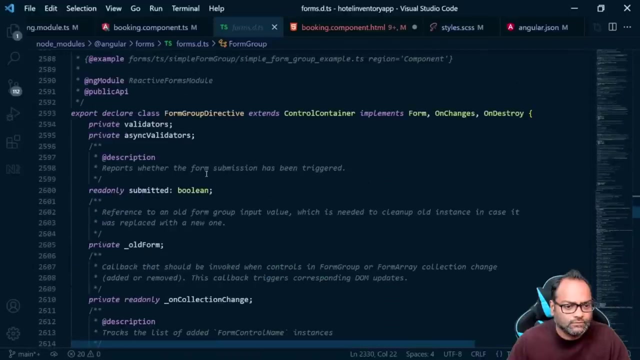 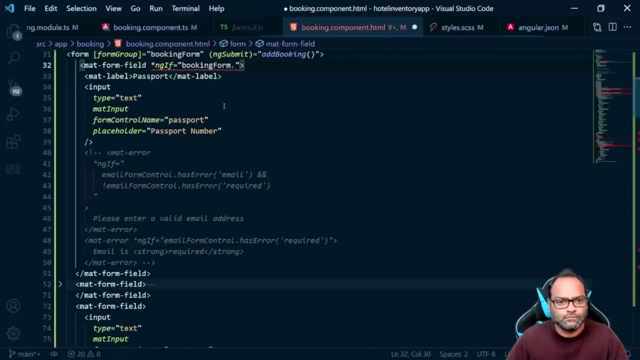 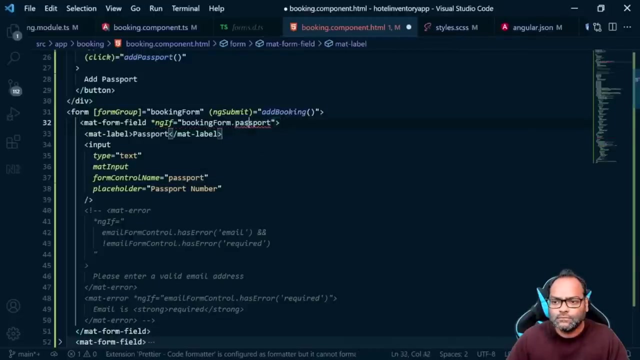 Sorry, not this booking form. Dot control dot. Okay, let's see which API we have contains that value. that value- Okay, let's see which API we have contains that value. Okay, let's see which API we have contains that value. 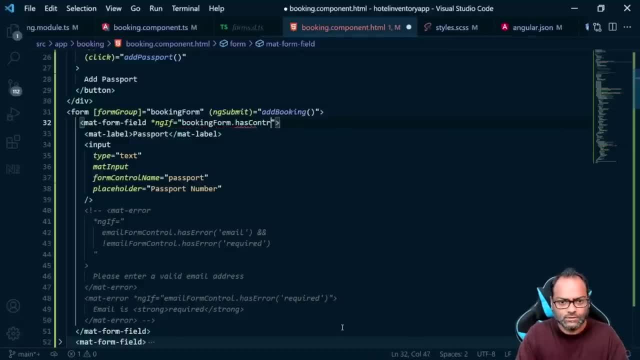 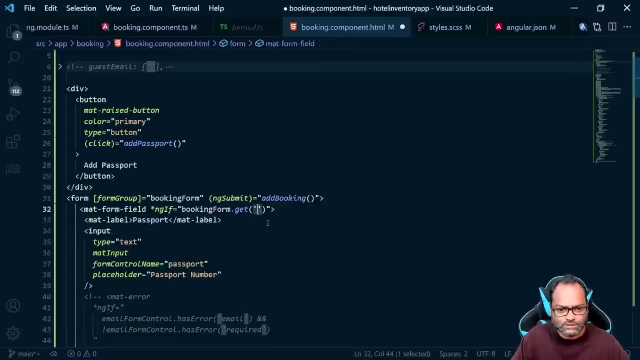 Dot minus control. Oh, here we can just check, get and put the control in. So we can use this get, So we can use this get. So that's where you get access to any video there. So this will Video game. Okay, so you can use these check to get access to any video. 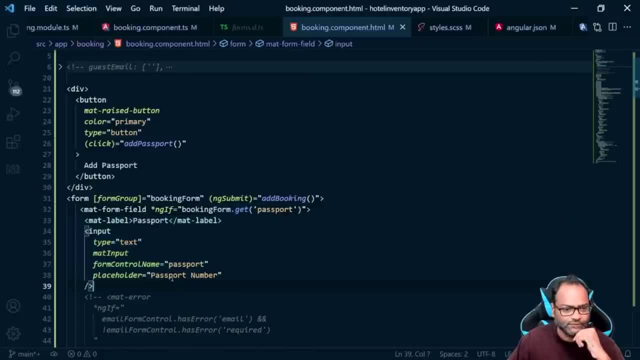 And if you want to view video games, you can use it for all other important things You can create bringing information. You can create inks tjos with Focus. You can create inks tjos with Focus. Check that all works. 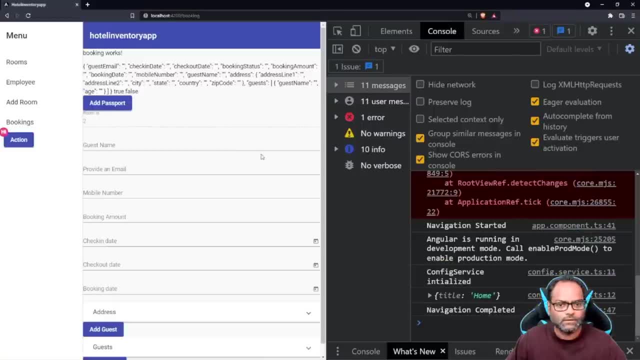 But otherwise, then another method to access to the contents of any information. So in case this particular control exists, then show, go ahead and show this, otherwise You have it right here. Check that. so in case this particular control exists, then show, go ahead and show this. otherwise, 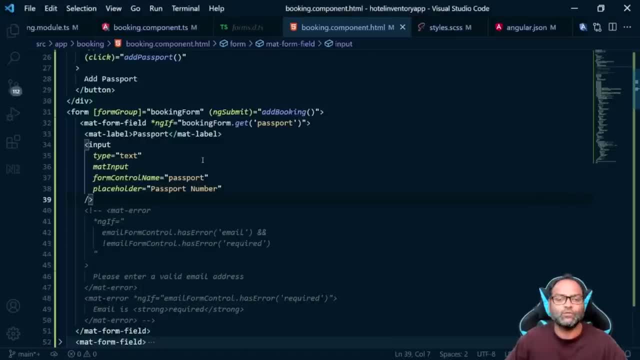 don't. So that's how you want to run it. And now we don't get an option, And now we don't have an option, a control dynamically, and you want to render it. adding is okay, right, we saw that. okay, we can just. 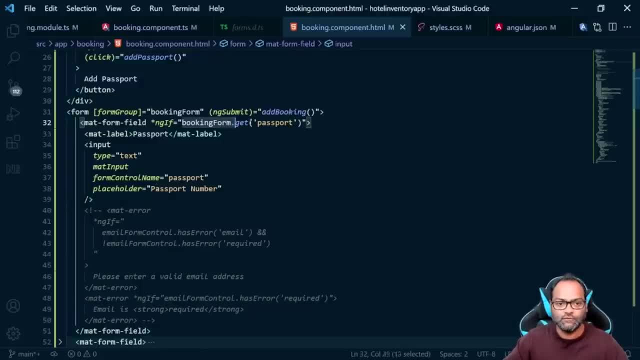 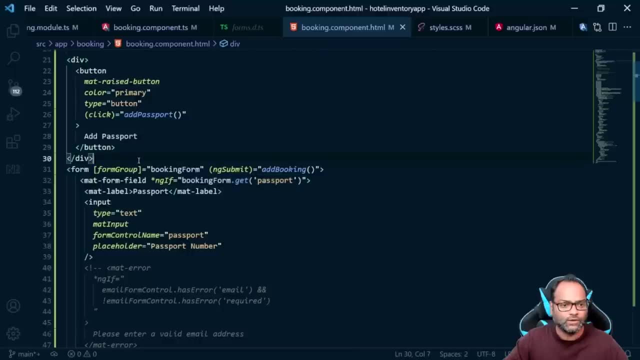 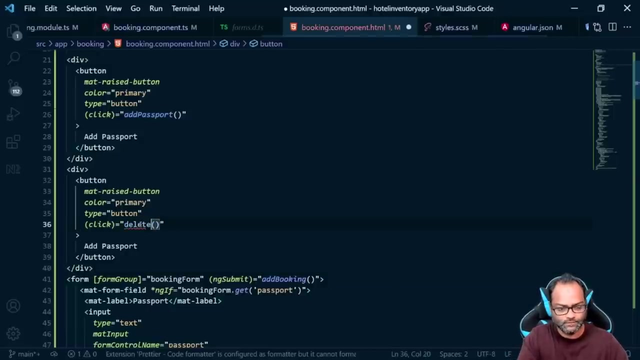 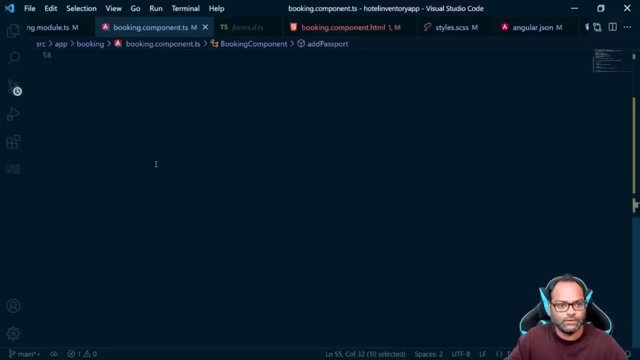 add it, but how to render it? so you have to go ahead and check first whether the control exists. if it exists, go ahead and then add the control, otherwise don't. so using this code you can also remove. i can say delete passport, and here we can call the other api remove control. so 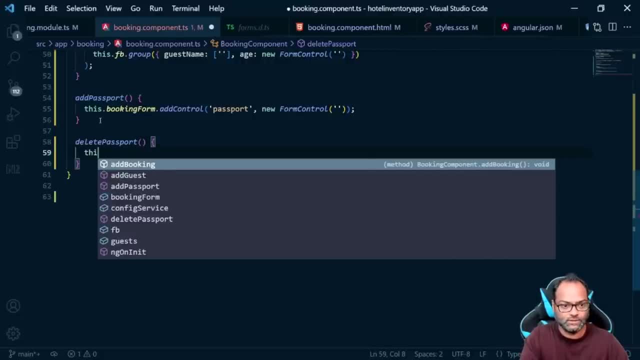 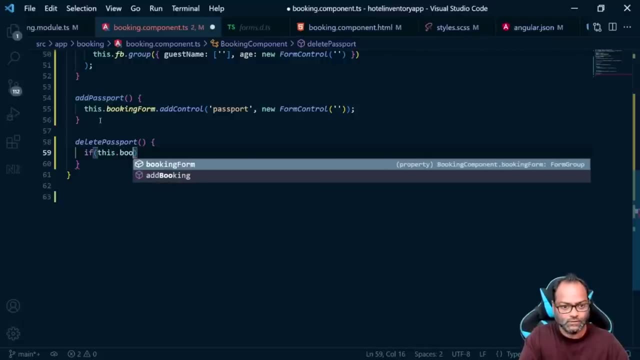 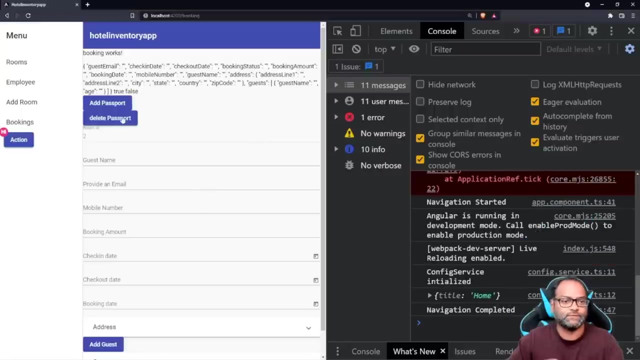 first i have to check whether the control exists so i can say if, if this dot booking on dot get the control name, uh, passport, then go ahead and remove the control. so let's see, and we have to save the form as well. okay, it is safe. so we have add passport delete. 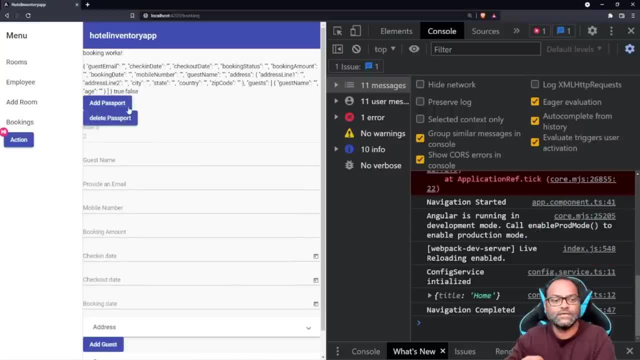 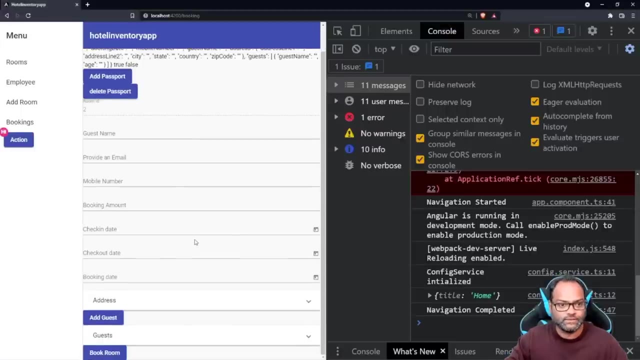 passport and the functionality works as expected, right? so you can see it's it. it's not like it's only getting deleted from uh ui, right, it's getting actually deleted from the form. so add form, uh, add passport, delete passport and we are done. one more thing, uh, as we are already talking about directive form or, sorry, dynamic forms. 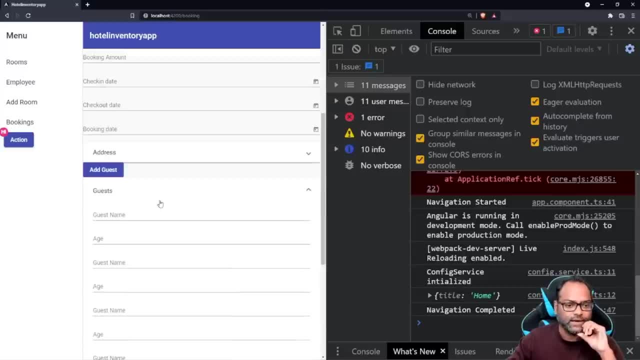 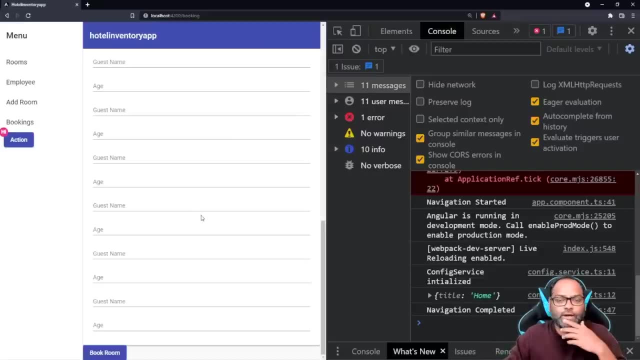 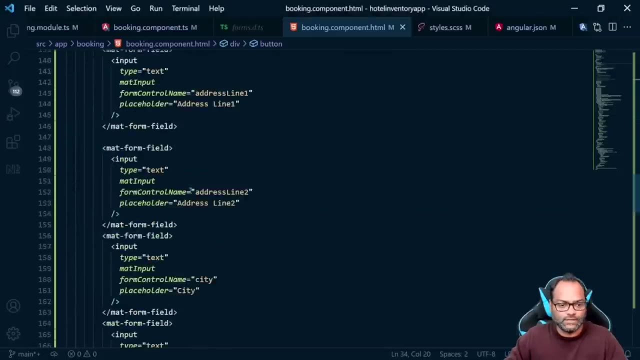 here also, right, we have multiple guests and we can add as many as want we want. but what in case? you want to delete what required? so we added one extra. what can you do? right now? nothing you can do. you probably have to reset the form. so let's see, uh, let's cover. cover this scenario as well. 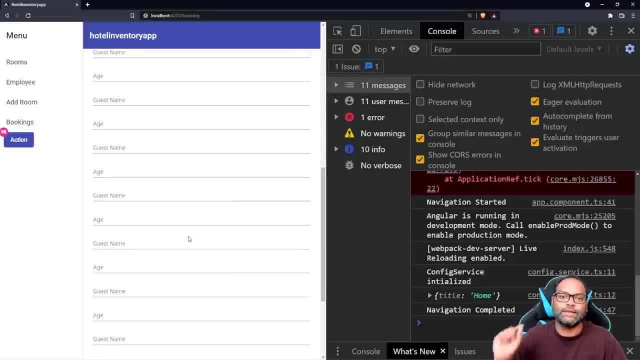 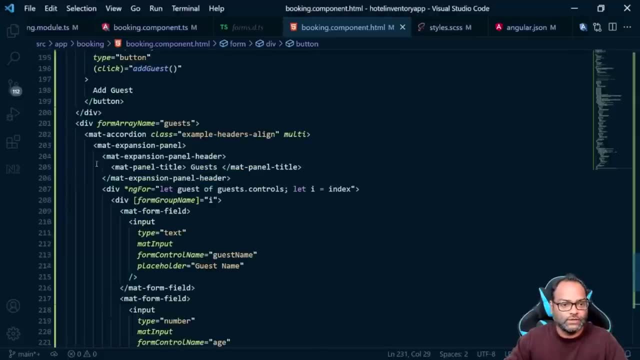 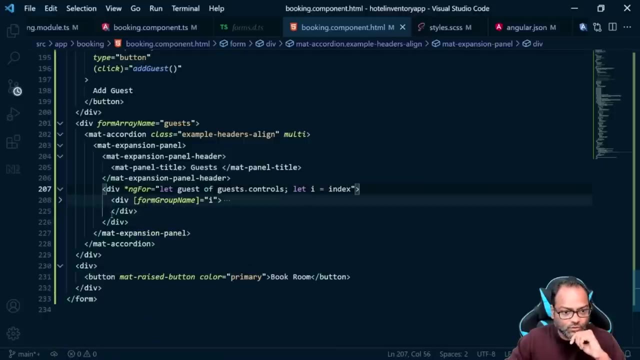 so to remove our control from the list of controls, we need the specific index from where you want to delete the control. remember this, keep this in your mind. so what we will do is: we need access to this form group. so we need access to this, i actually, so i have to. 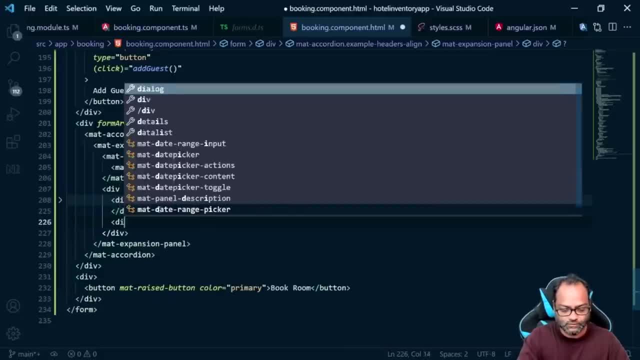 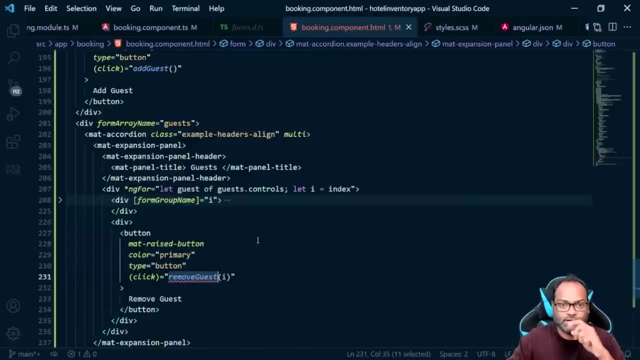 add this button inside this div. so here we'll add one more div which will say button and i'll say remove guest. uh, so this is remove guest button which we have added and let's implement. and we are passing this side, we are passing the index, from where we want to remove the control. 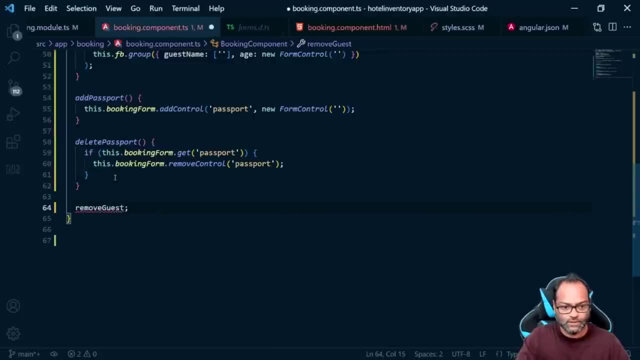 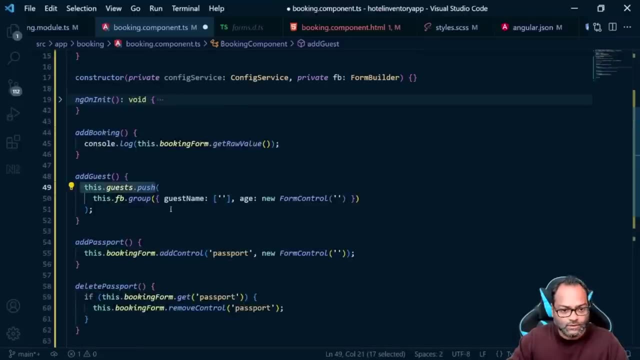 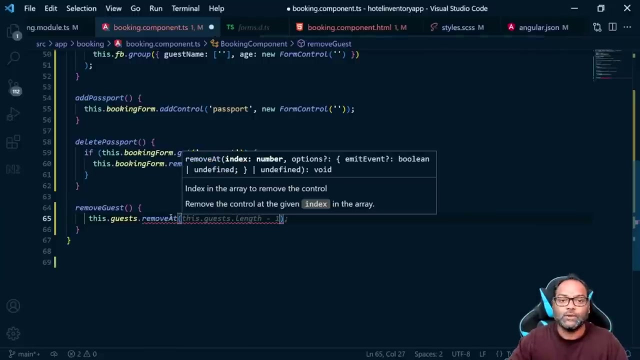 so here i, we can go to remove guest and yeah, so we can just do this, dot guess, dot, uh remove at. so we can pass the uh, pass the index which we are receiving in this function. so we are saying i, which is our type number, and we'll pass this index here and 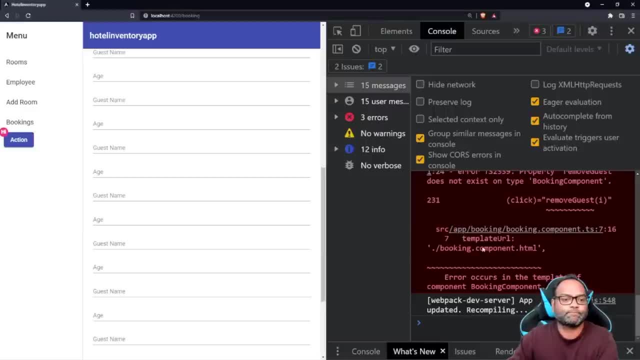 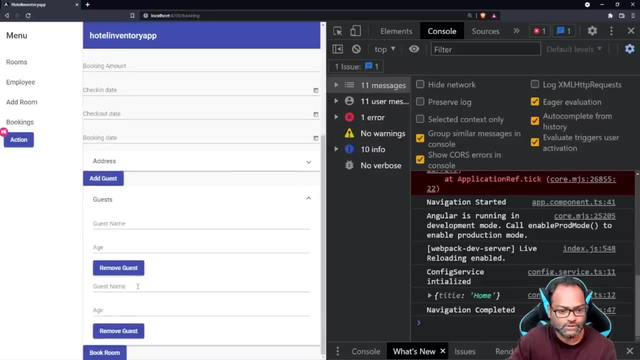 the control will be removed from the array. so every uh row- so here we'll see every row- will have a remove guest button. so as we add one more, add one more and it remembers from which index it is removing the control, right? so if i remove, let's add some text here, and if i remove this one, it remembers that i had removed one, the first one. 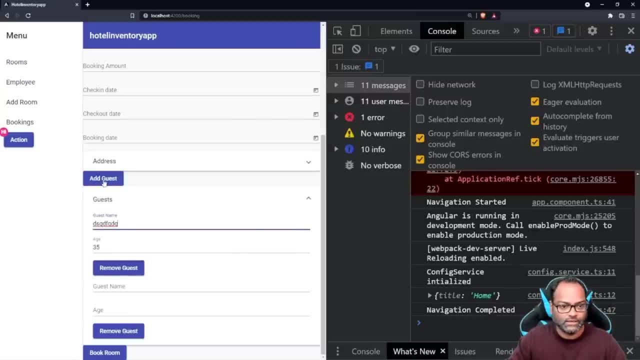 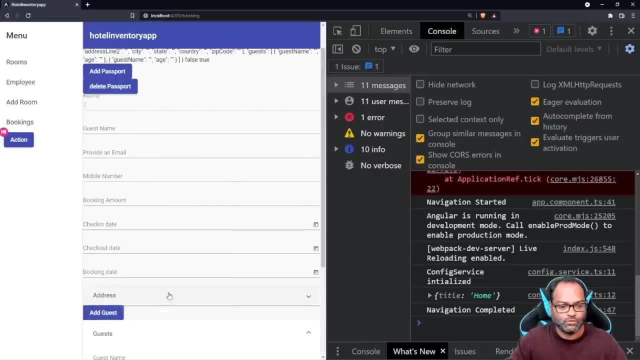 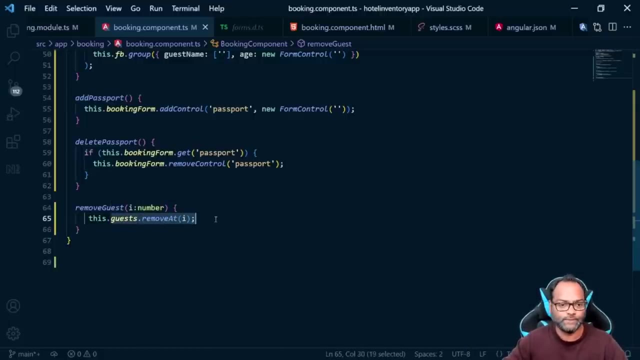 so it will not change the values, remember this. and you can add one as many as you want and then remove as many as you want. you can remove all and then add more. so this is how you can actually do dynamic stuffs with this particular api. so what we learned? we learned about the form. 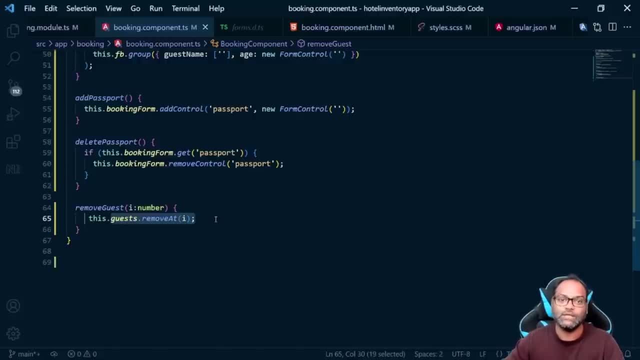 array. we learned about how you can add multiple- uh sorry- controls dynamically using form array. then we also learned about how you can add done controls dynamically using add control, and then you can remove them using remove control. and then, similarly, we saw how you can remove controls from. 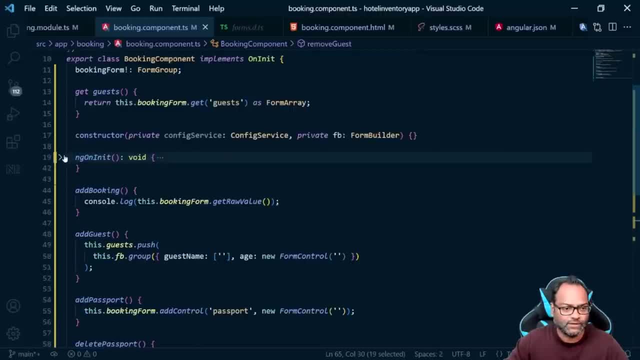 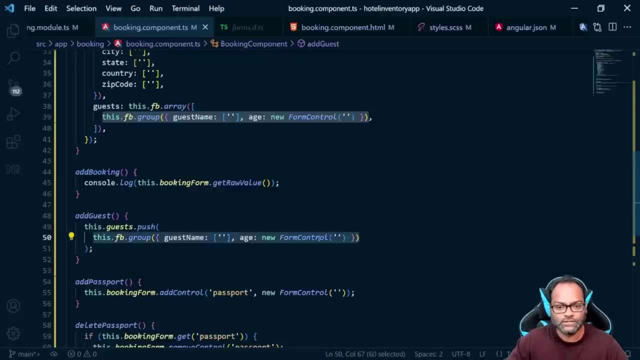 an array. one more thing: uh, you might be wondering that, okay, this code and this code looks same. yes, they do look same. so what we can do is we can actually go ahead and export this. so we can just go ahead and say: right factor. and we can say: 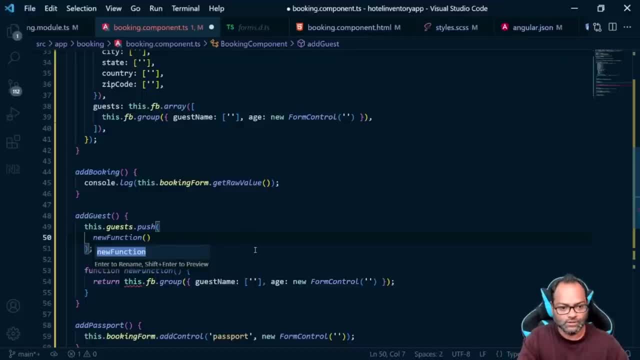 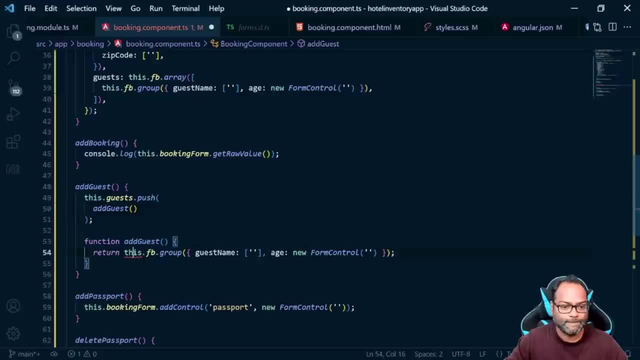 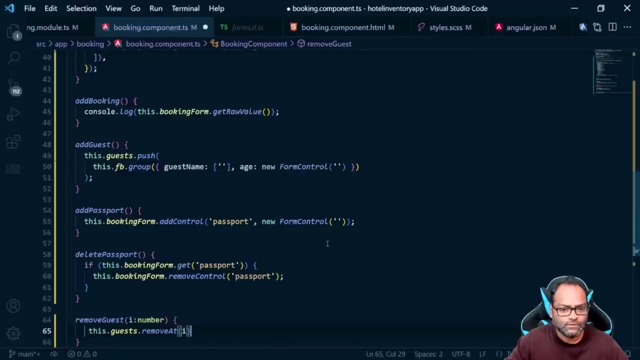 let's create a method, let's create a function, so i'll call this function as add best. okay, and let's see, okay, somehow it got added inside this for some reason. okay, something wrong here. i think i had guessed functionality exists and i just named it the same. 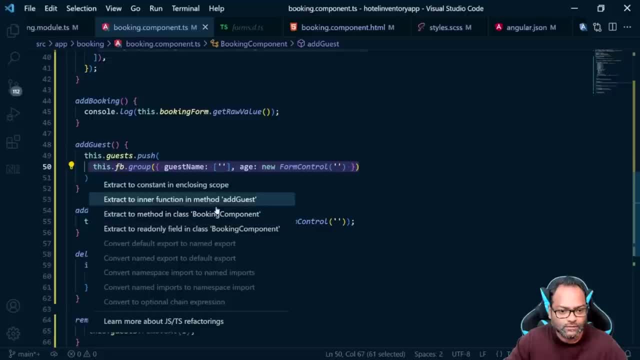 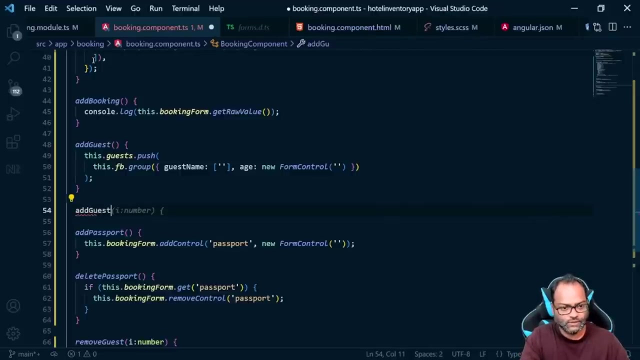 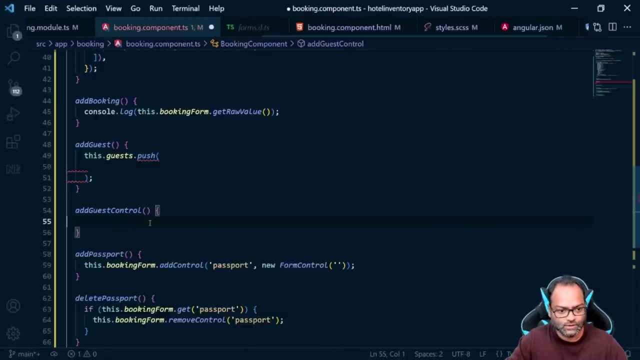 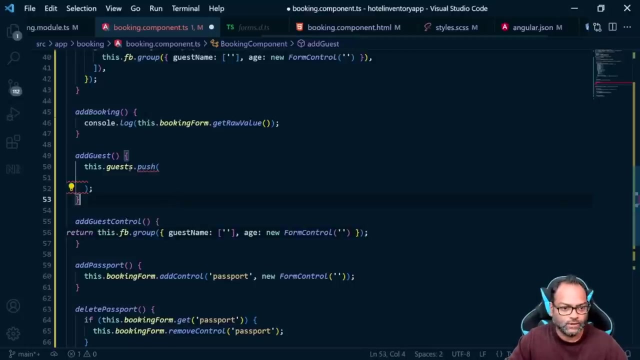 so we'll say: retracted. uh, accept to inner function in method. no, i want to actually extract it in the function. let's write it, not problem, add the guest control. and here we'll just use this code and we'll say written: let's not try, and here we can add this dot: add guest control. 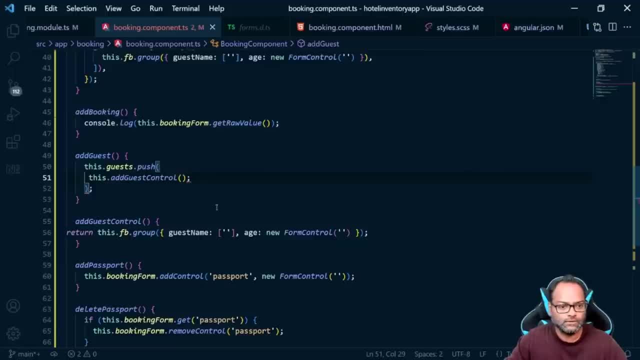 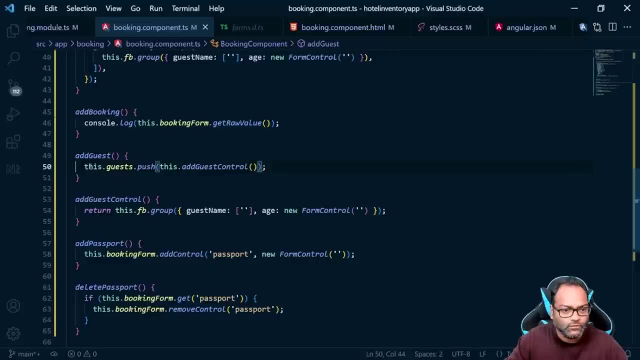 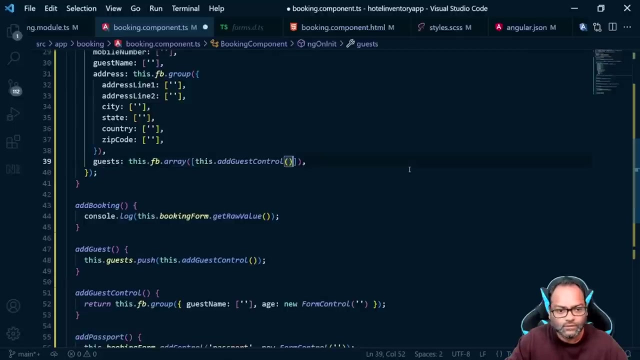 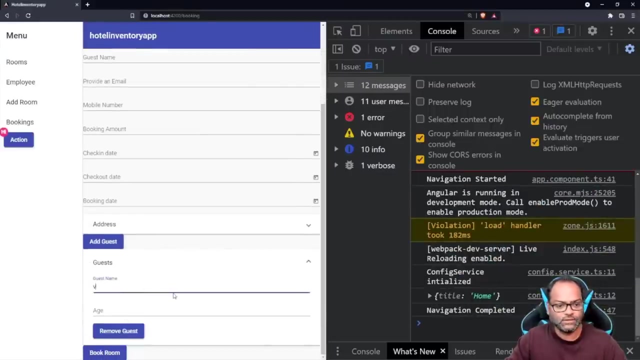 and similarly we can, let's format, we can use the same line, this dot and guest control here. let's verify so we have. we don't have any errors. the guess is available here. let's add and see if the value is available here and it is. and let's 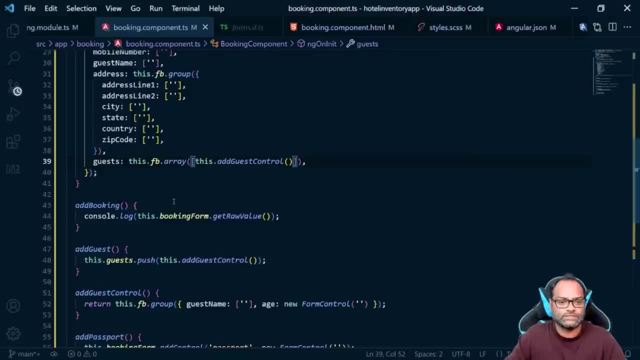 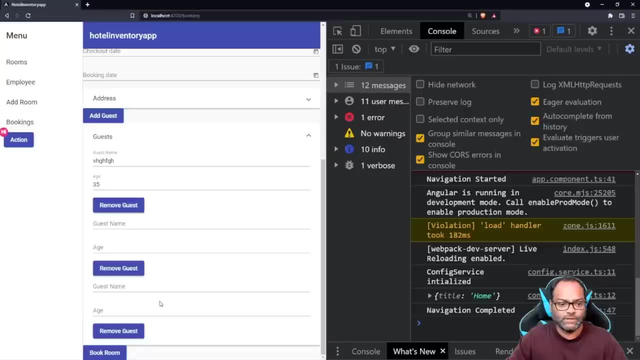 click on multiple guests and that's it. so we don't have code duplication as well now in this particular code base. now, what we will do next is we will add some validation. right now there is no validation. we completed our form. we wanted, uh, we want. we added all the controls which we needed to create. 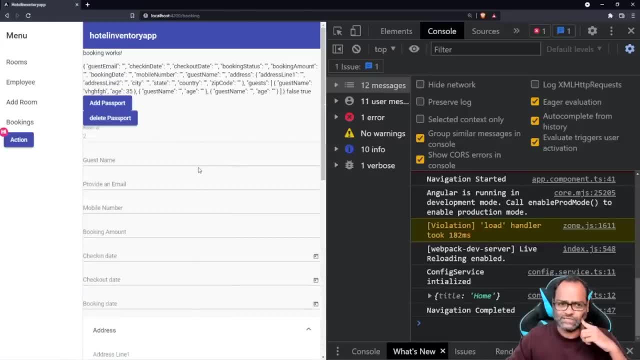 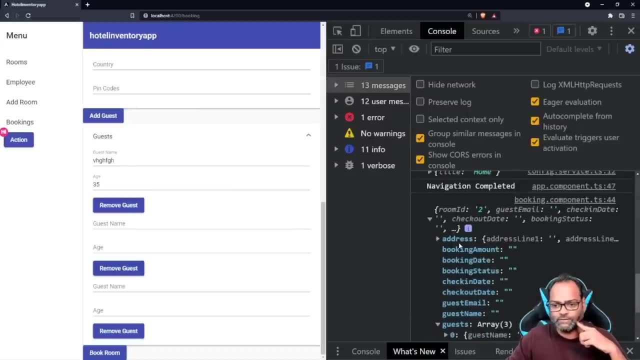 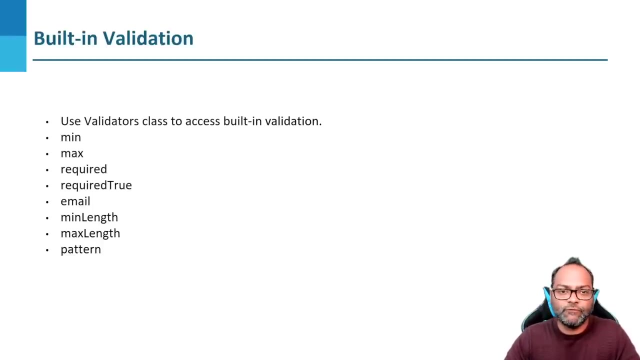 a booking form and uh, let's square and add validation now, because, you can see, i can just go ahead and submit without anything. and uh, you can see, uh, it said: it's all empty values all over there. now we will add the validation to our form, but right now we don't have any validation. so 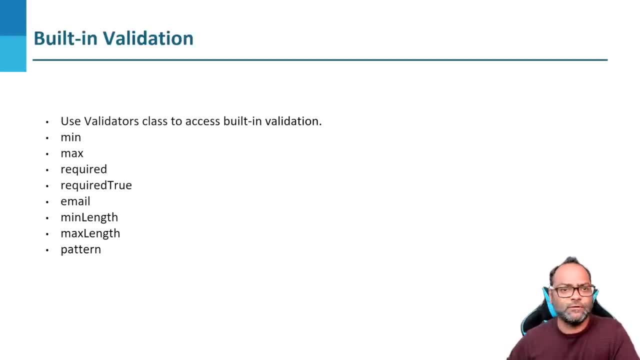 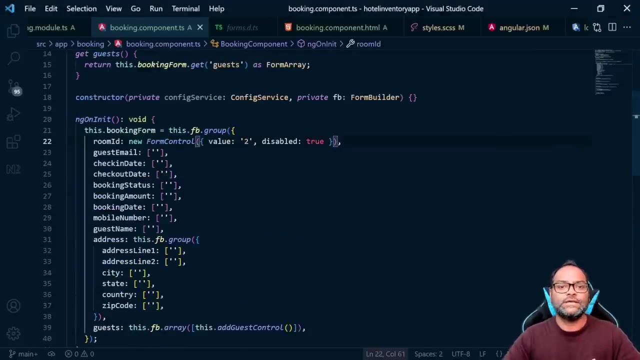 let's see how we can add validation to reactive forms. we have already learned it for template driven forms, remember, we can just use html5 validation. so in a case of- sorry, in case of reactive forms, let's see how to do it. so it is actually a second parameter which is available here. you can see, uh, you can see the. 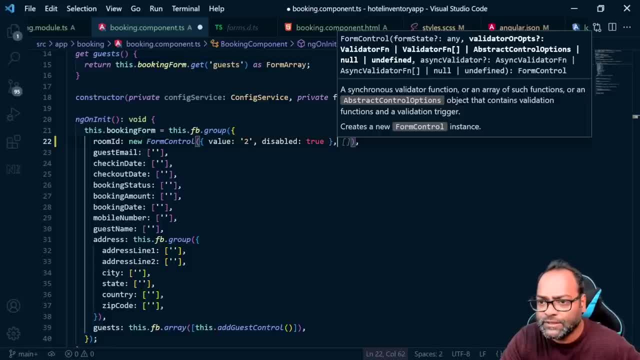 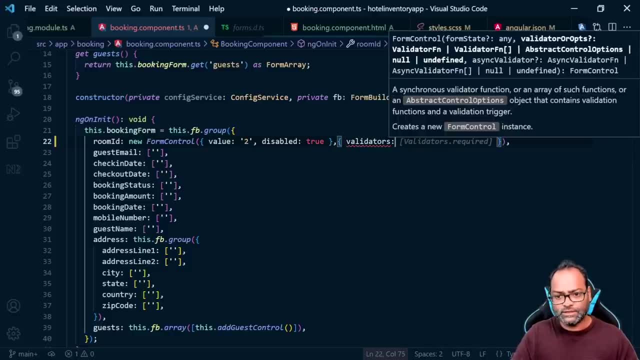 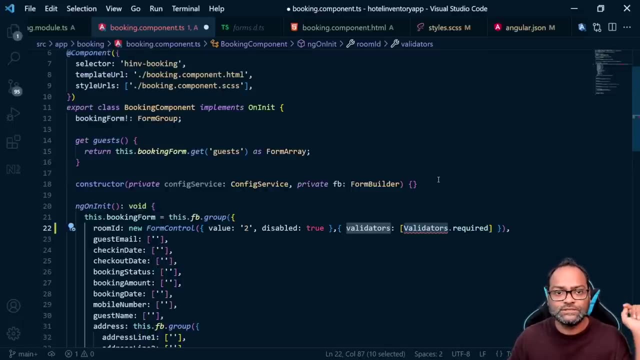 typings. so it says: uh, the second parameter is validator or options. you can actually pass it something like this: you can say validators and then there is a class called validators. remember, validator was an interface which we used in previous video while talking about adding a custom validation to a template. 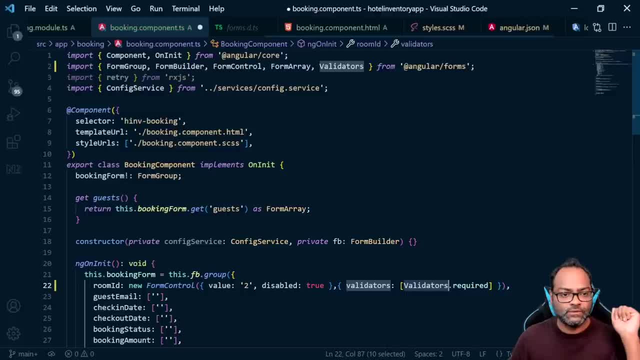 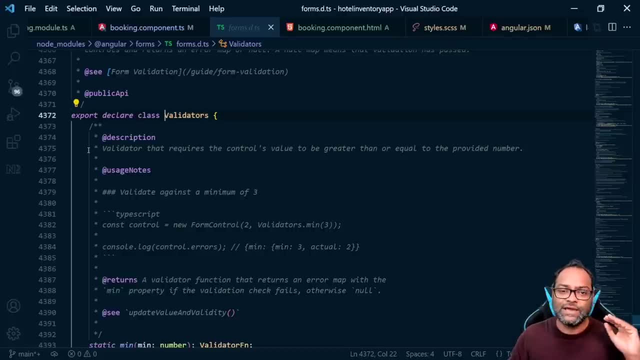 so we have a class called validators class, which we have in html5, and it's class is called variable class and it's class is called variable class. here we are talking about a validators class which comes from angular slash forms and it has all the validations, built-in validations- which 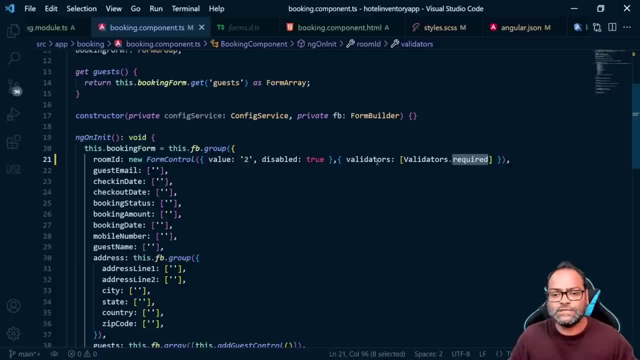 we have seen in html5 validation, so you have min max required everything. so let's see how to use them. so here we are saying, okay, validators, validatorsrequired, and similarly you can also add it here: two validations here, which is validatorsrequired. and then we are also using email, else what else? 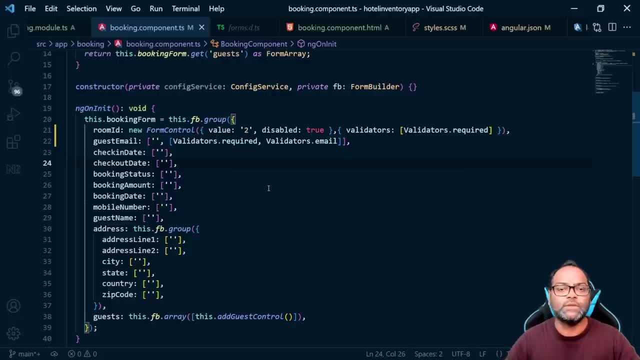 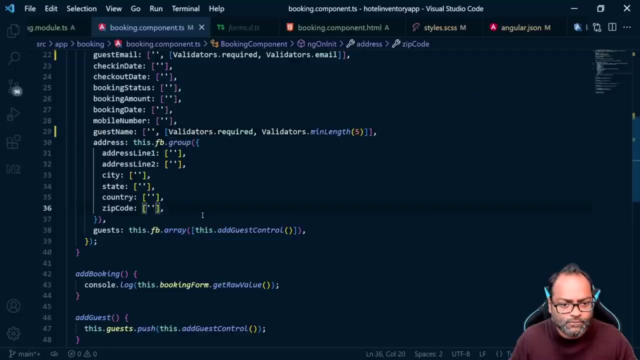 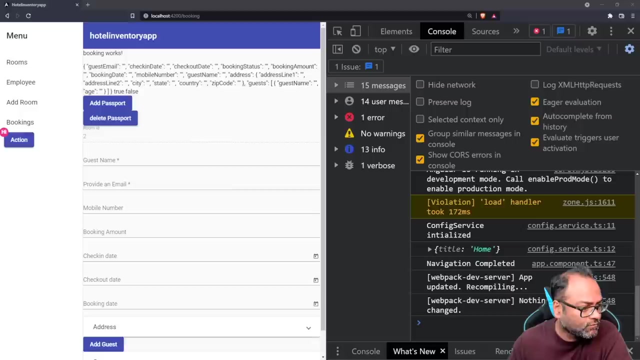 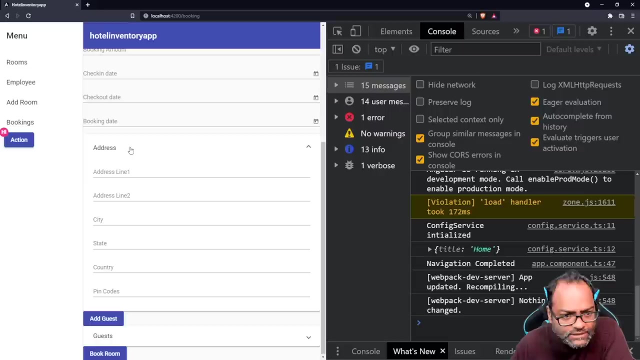 we can apply. you can also play with min max. so let's check. we can have guest name as validatorsrequired, and then we can also have a min length of five, and let's go ahead and see our form. so here you can see a star. so at some places or some properties, you will be able to see a. 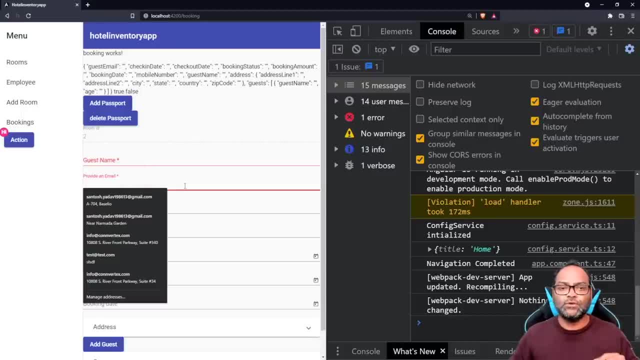 class available here. sorry, a star available here. it's actually. you don't have to do anything with angular material. whenever you add validation, you will. also, we will get the star when it's default behavior and it tells you that. okay, this form is not valid right now and it's easy to figure out. 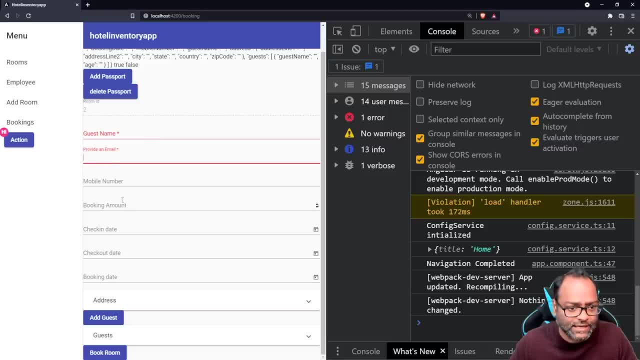 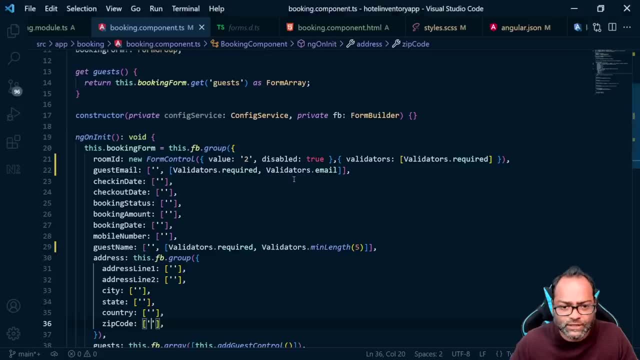 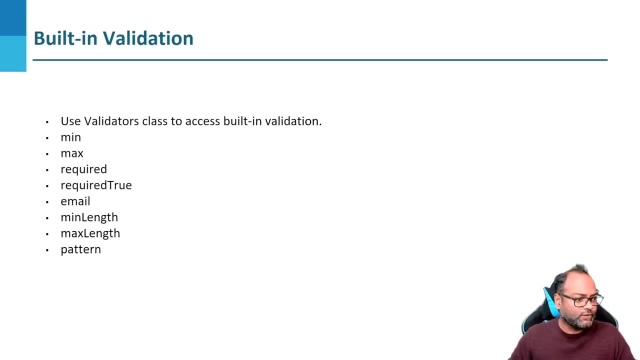 the validation error as well, right, we added it for guest name and email and for room id, right? so which is already true, and you can add more validators as you want. so the validators are different type of validity validators which we have has been matched. required, required, true, so i 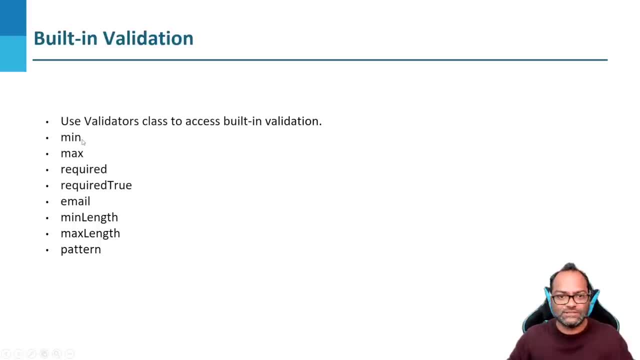 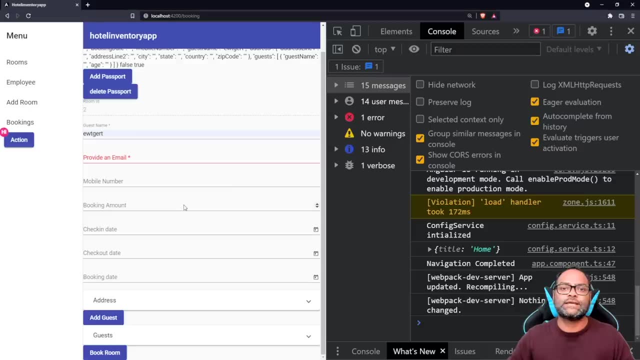 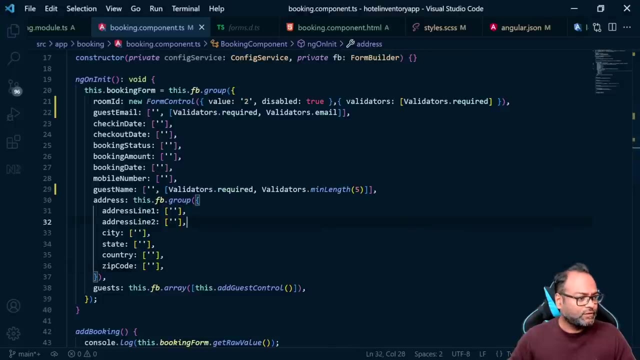 mean i'm sure you know, uh, the others, because they are same as we discussed about while working with template driven forms. let's see required true. so for required true, it's like let's say, if you have a checkbox, right, so let's actually add a checkbox, and we will go to material and we'll see, uh, how checkbox. 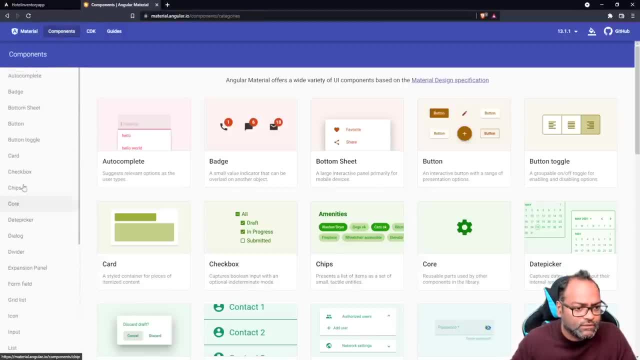 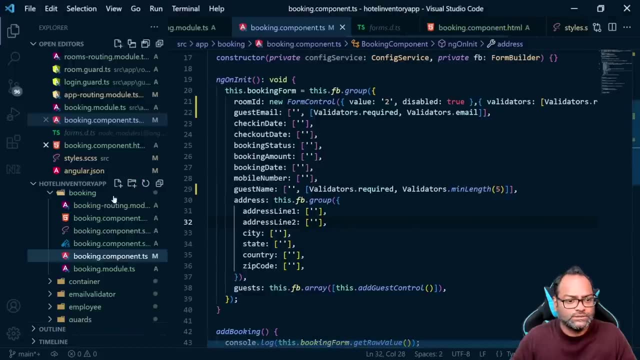 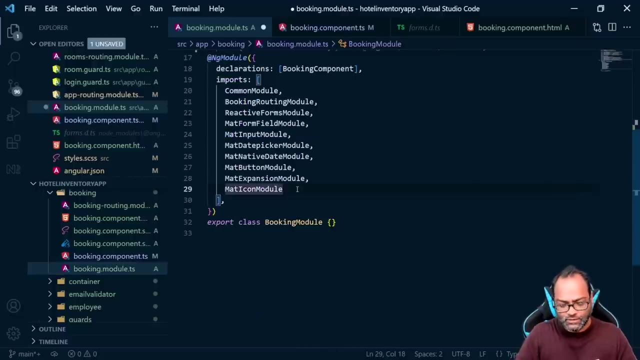 can be used. so here, uh see, so we have a different api for max match box. let's add this: remember why the reason i always refer, that i'm referring to the documentation is to make you an habit of referring to the documentation whenever you are working with. 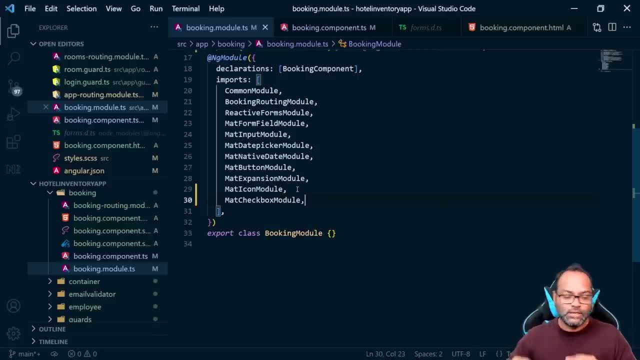 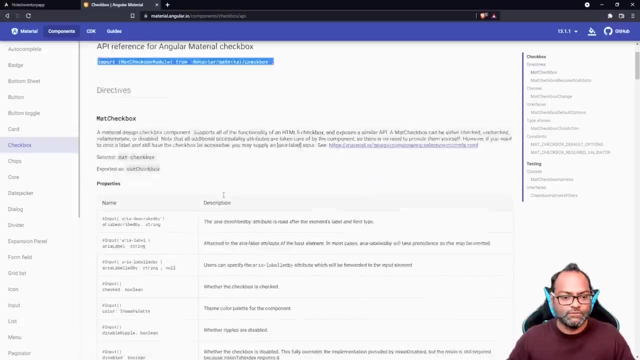 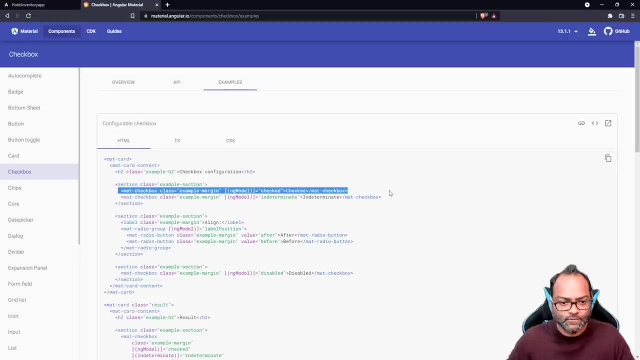 any ui control, because there are chances that in some- uh like in next release, they can add something extra and if you get into some issues, you will be able to easily figure out that issue while by using the documentation. so now we have this checkbox available, let's go ahead and add a checkbox, so we will say match checkbox and rather than 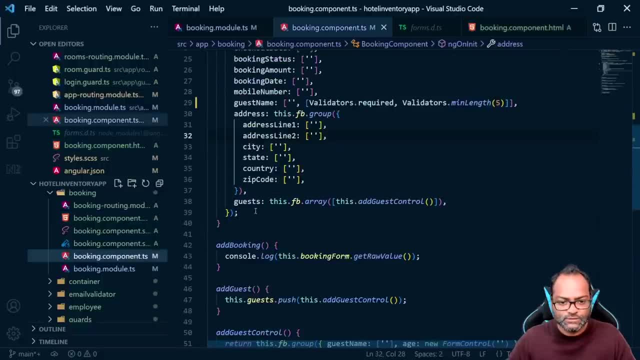 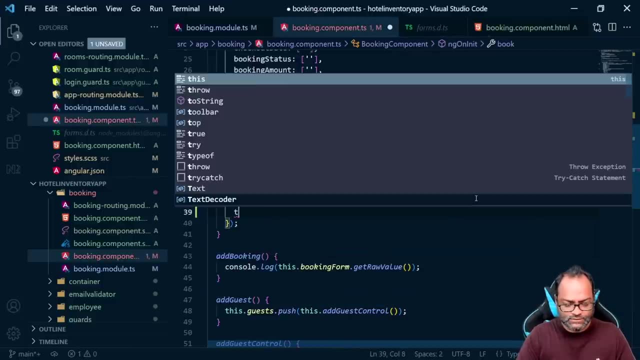 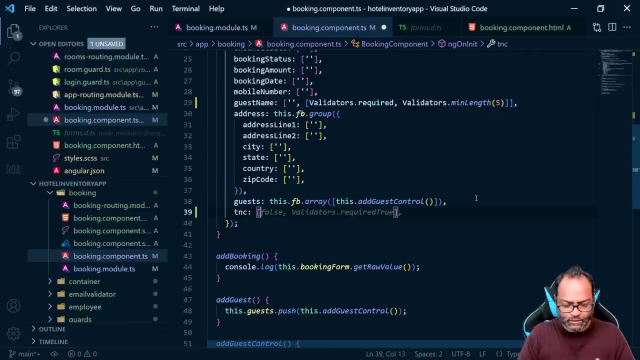 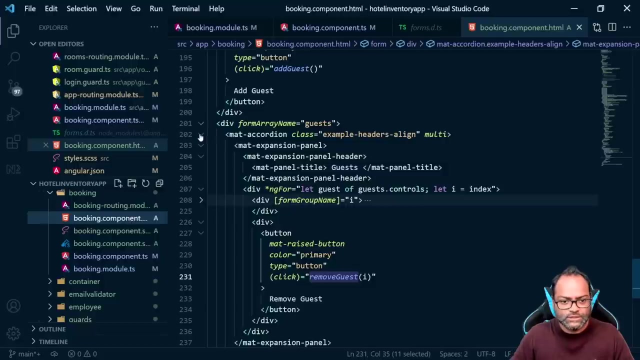 using this. let's add a property first and we'll say: this is uh, pnc, right, so terms and conditions, which is new form control, and we'll pass false and then we'll pass required to. so, before you can proceed with the form, you have to submit or select this tnc, so we will place it after this. 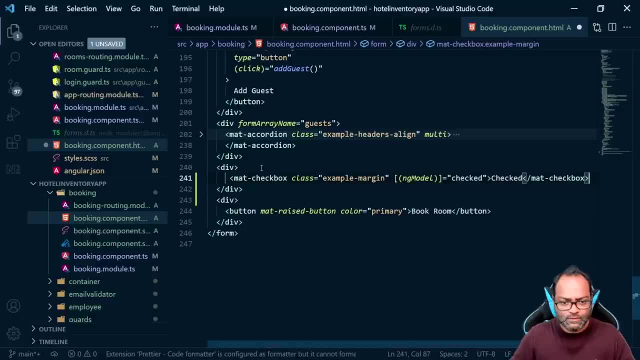 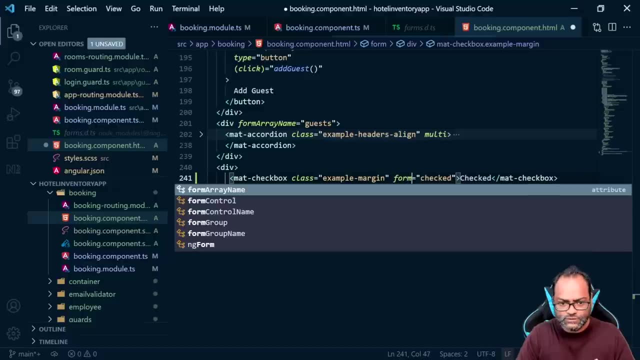 match check box. we will not use ng model. so we will not use ng model, but we will use the match check box. so we will not use ng model, but we will use the match check box. so we will not use ng model, but we will use the match check box. 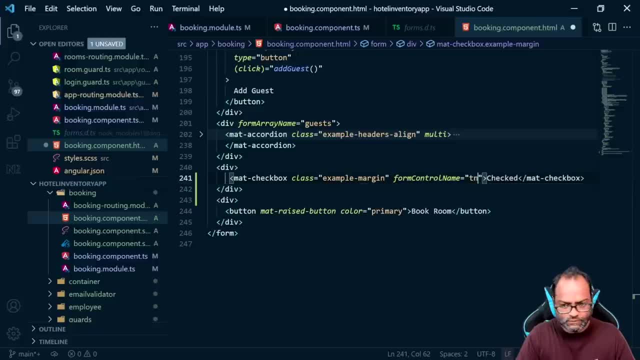 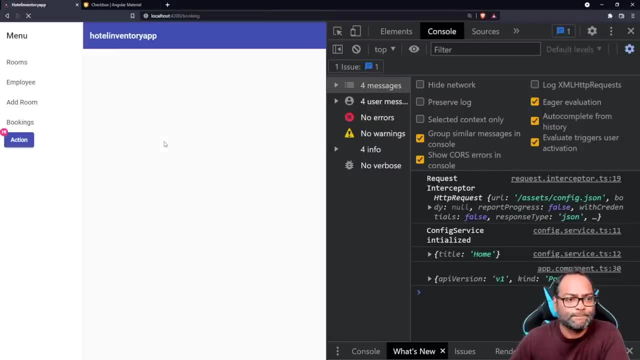 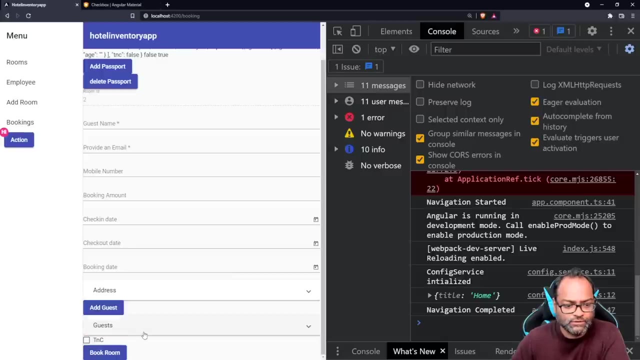 control name, as we saw, and we will say: this is tnc- tnc terms and conditions. let's see, so you can see. uh, you have this checkbox available here now, so we have to check this, check this box, uh, to proceed with, i mean, uh, to proceed with submitting the form, but we have not added that. 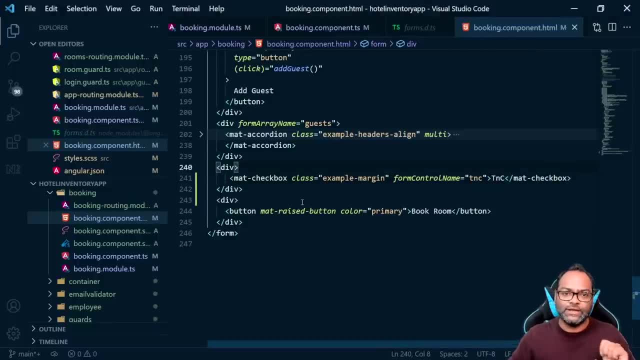 check as of now. let's go ahead and do that. so we now add some validation, but our form is still. we will be able to submit our form. so let's use the same approach we used earlier. so we'll say disabled and then you can say: this is booking okay, somehow. 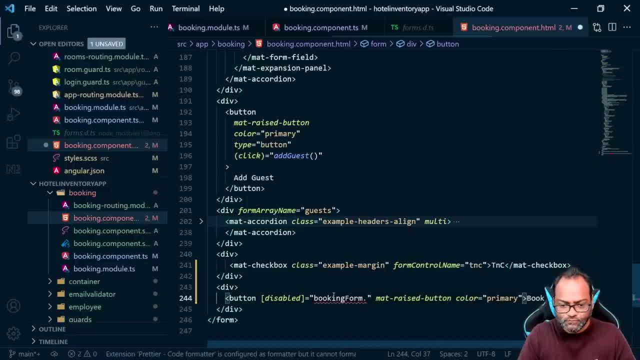 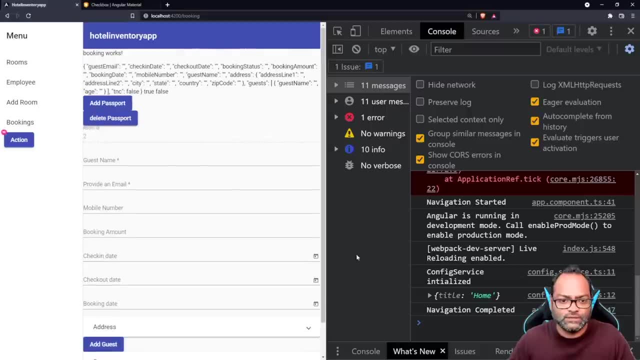 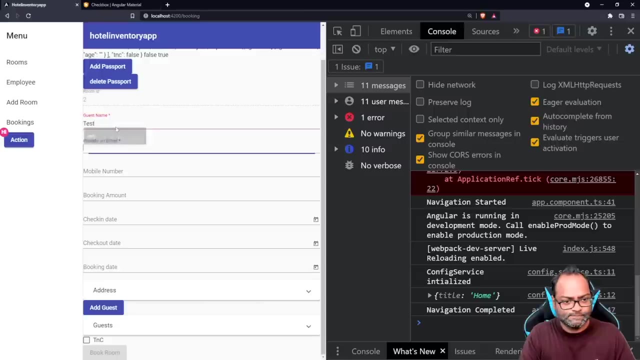 typing is not working for this dot, keep it disabled in case the form is invalid. the same things, the same controls are same properties are available here. so now you can see the book room is valid. let's provide all the values, mobile number, i mean. these are not required values, so we'll just move on to tnc and 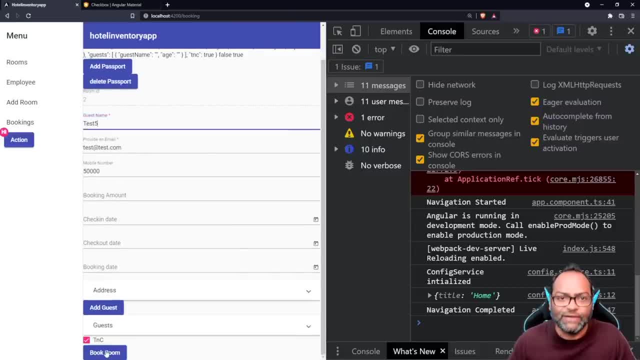 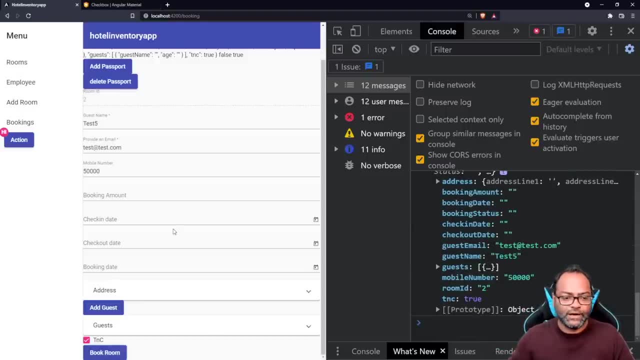 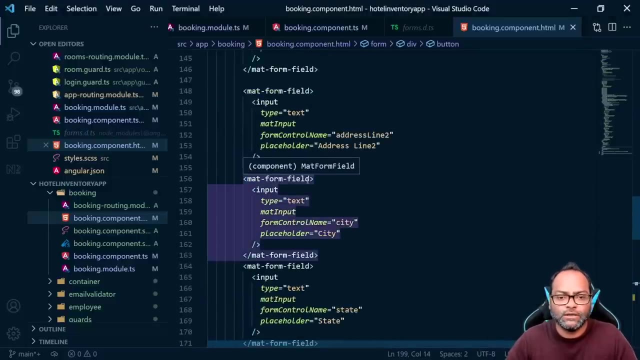 okay, guest name should be five character and you can see the button becomes valid and you can click it now. so we have some validations in place and we have added a required brew validator as well, and Now you can play around with other validations. So you have in max email we already added. 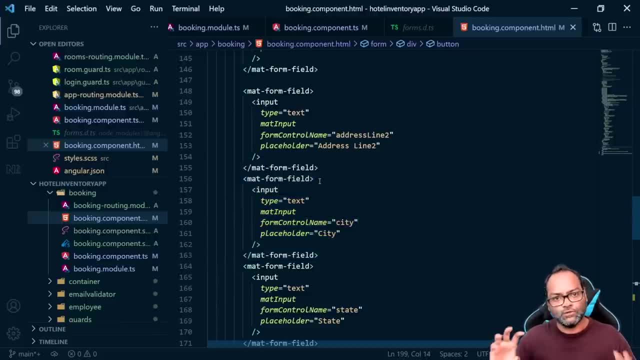 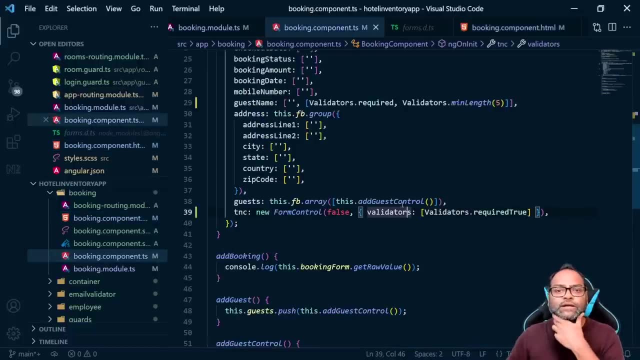 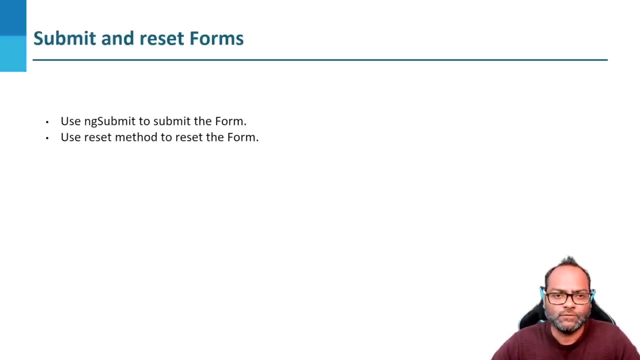 We have pattern. in case you want to have a control, where you have some regex, You can also apply the pattern property as well. So these are few built-in validators, and now let's move on to creating our own validator. Before we learned how to submit the forms, we also added the validation. 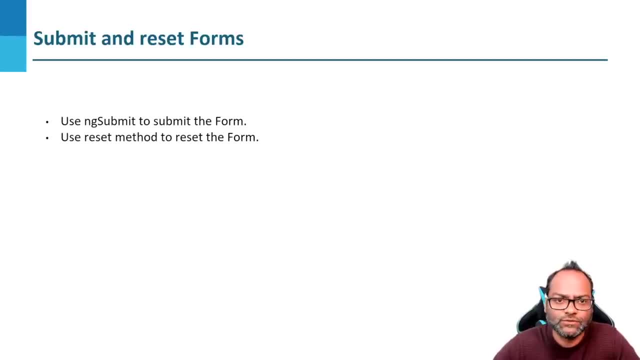 Now how to reset, right, So we have not seen that scenario. so, as of now, We know how to do reset. We already learned about it. If you remember, we did it for template-driven forms, So let's go back to the code and see how we can do it. 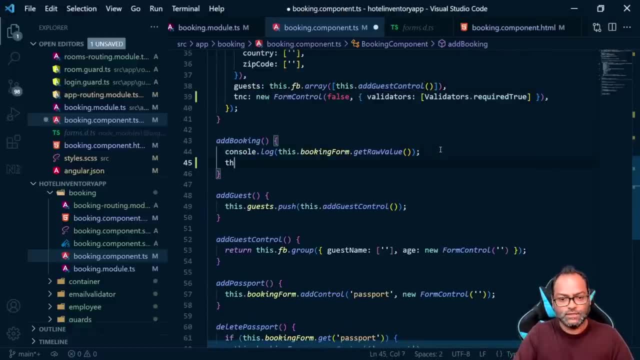 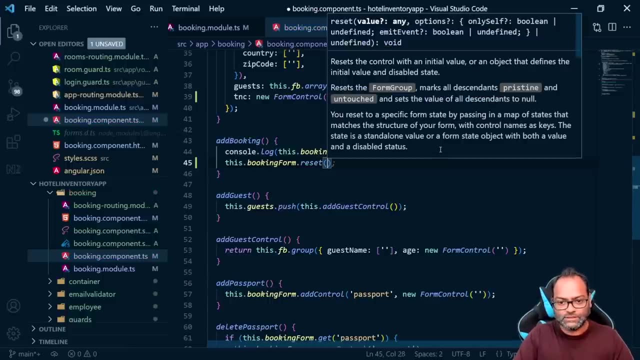 So we will go to our add booking method and here you can do something like this: So this dot booking form dot you can call reset, So you can see you can pass all the values. So its value is optional, So by default it will just make every. 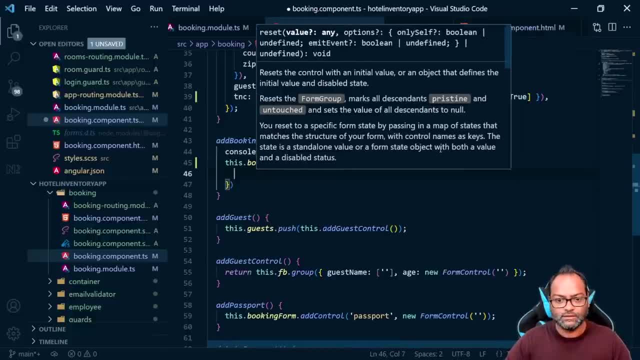 You can call the set so you can see. you can pass all the values, so its value is optional. So by default it will just make every to null, which we don't want to. so you can provide the values for each and every control which we 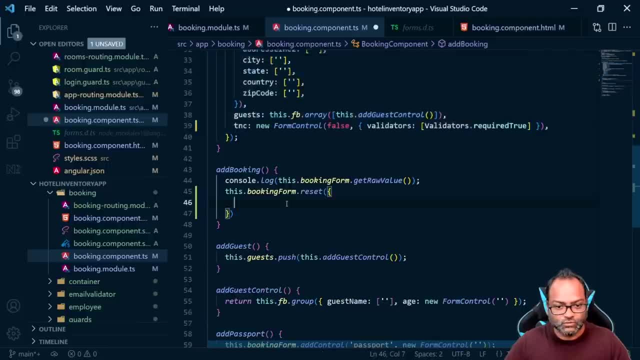 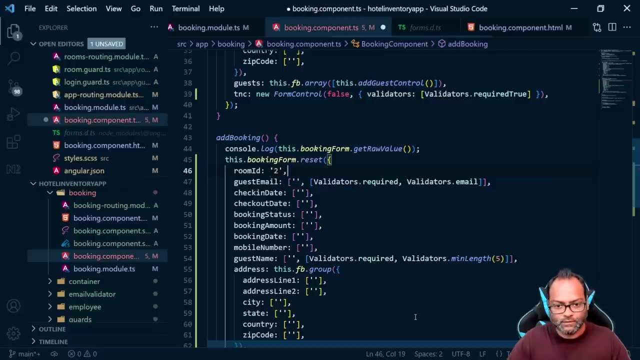 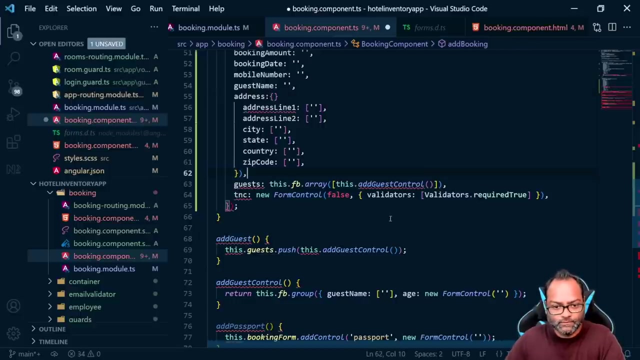 have available here. so let's do that here. so remember we are providing the values, not the control value, right? so we can just have the default values for each and every control and this is guest name here. we will just remove this and put a curly bracket. so. 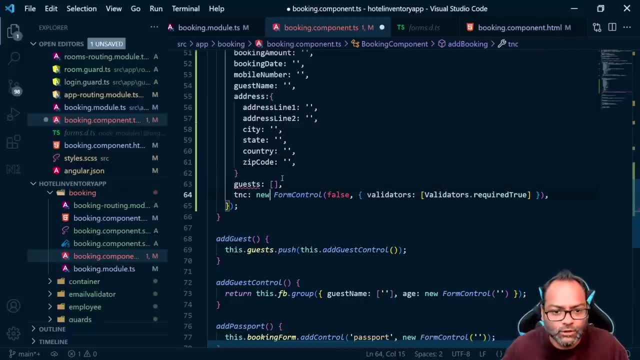 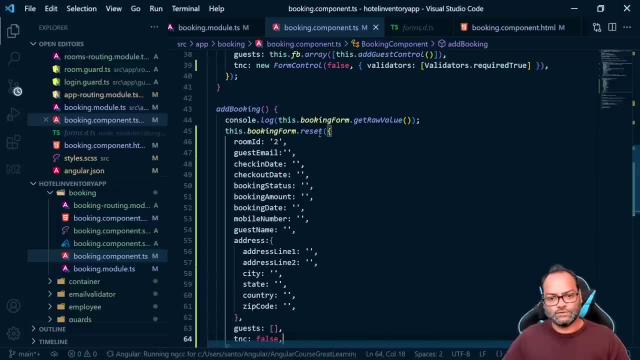 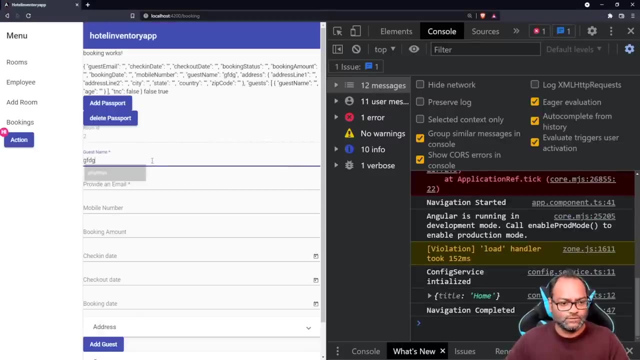 here we can just pass an empty array. we don't want anything to be available, and in tnc we can just say false, so let's go ahead and verify. so we are using reset method. let's provide the values so we can say: okay, this is tom. uh, we need five characters, so let 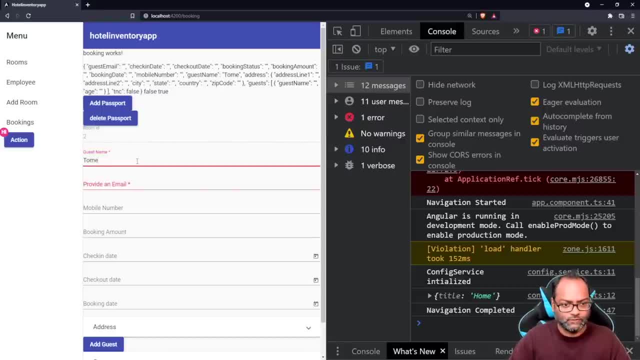 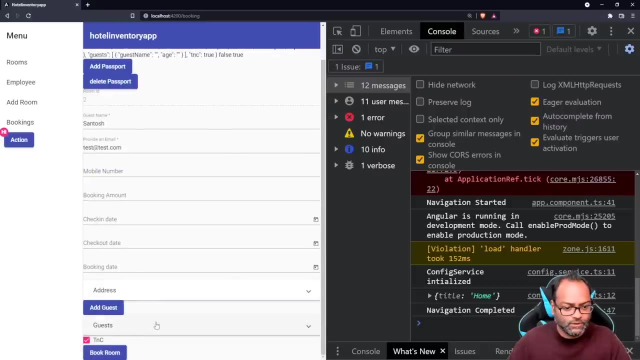 me just enter my name. okay, i just spelled my name down, okay, uh, and we'll just use the uh values which are required. right, and let's do that, let's save it and you can see, now the values are actually the same as the default values, so we can just 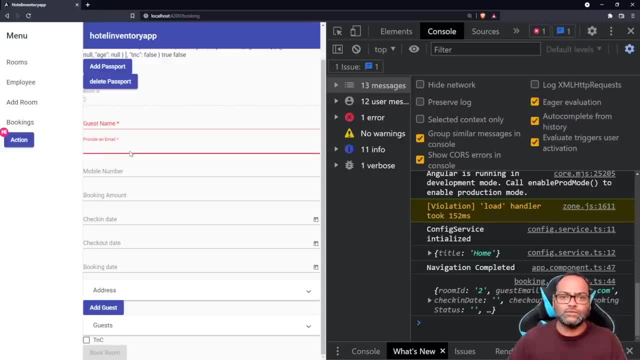 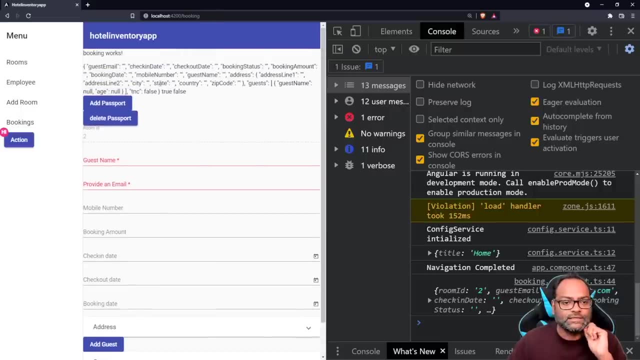 use the default values for each and every control. it's back to the original state, so we don't we have like default values available here right now, right? so whatever we pass, so you can see: uh, tnc, let's say tnc. tnc is false, guess, as we said, it's an m? mtr address. again, we pass some default values and this is how you can. 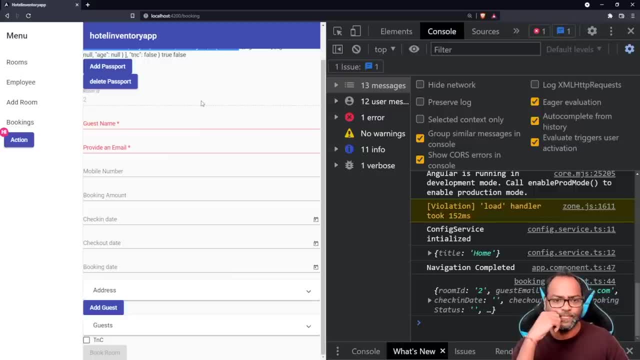 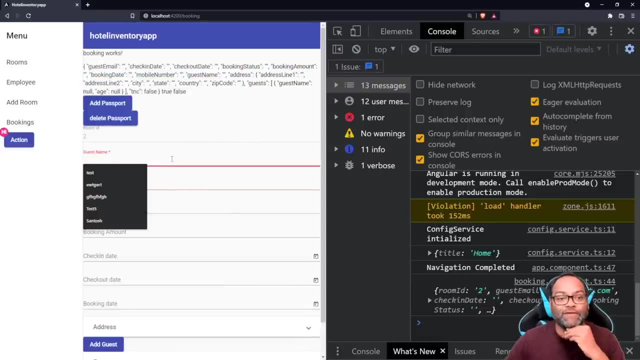 reset the form. one thing which we have not seen so far is what? what is missing? what do you think? so we have not seen how to uh validate the controls, uh, sorry, how to show the errors on control level. remember, this is one thing which we did: it uh, with template-driven form. 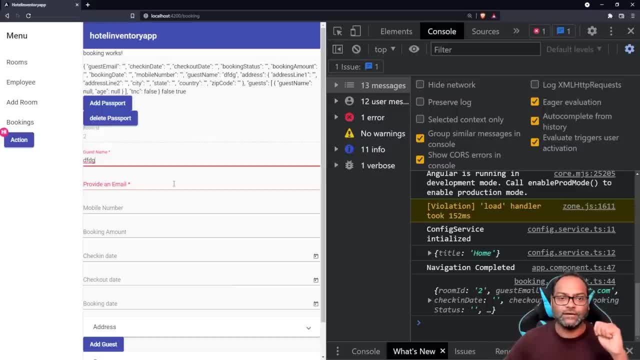 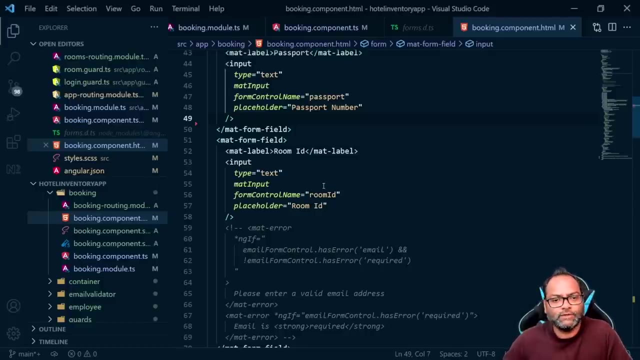 here, for example: uh, the guest name is required, but it also has a limit, right? so it has a max min length property which says it should be at least five character. so let's go ahead and see how we can actually add those validation messages here. so, uh, now let's see how we can add control level validation. we already have some code. i believe here, so we'll uh uncompage. you can add some code here, all right. so we just want to go ahead, and so we'll uh uncompage here. all right, so we'll uh uncompage here. all right, so we'll uh uncompage here. 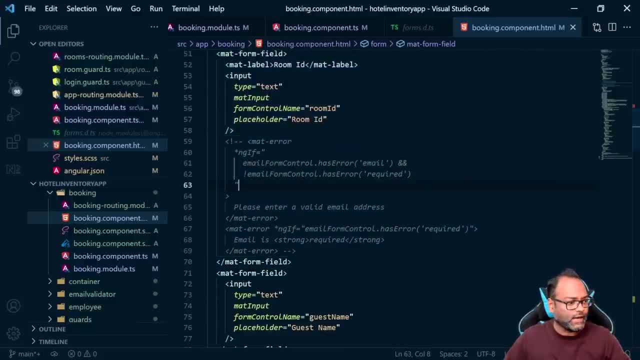 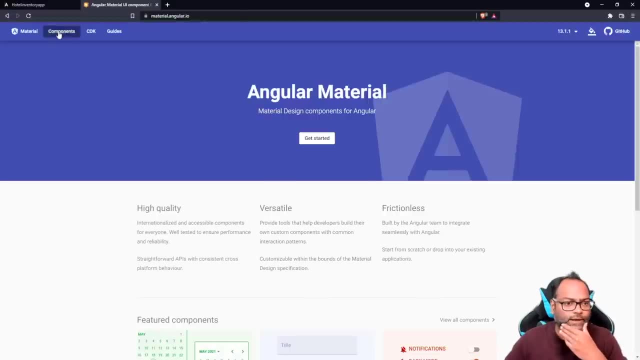 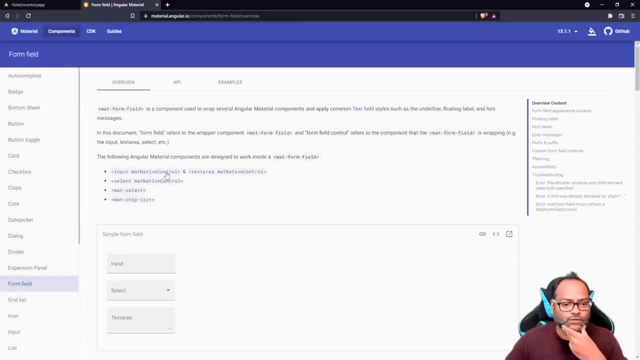 Uncomment and we will talk about it. So let's see, Angular material also has something known as mat error. So if I go to materialangulario and components and let's see, is it's part of form filled and you can see it's, and there should be an example. this one: 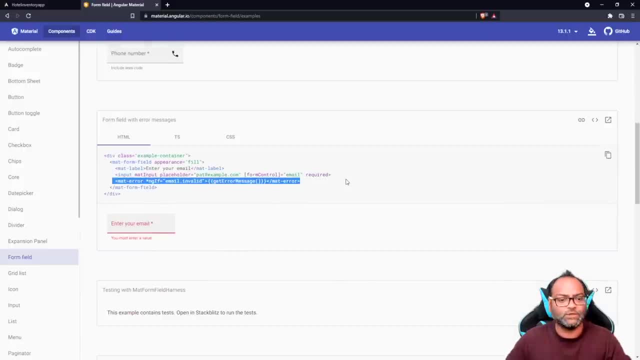 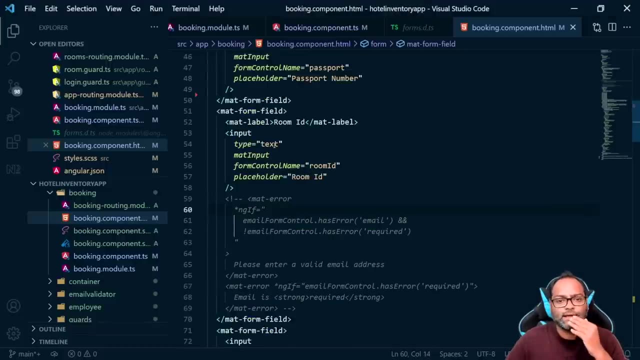 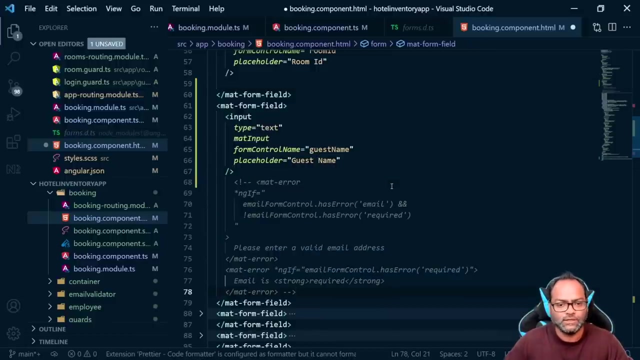 form filled with error messages and it has something called mat error so, which we are going to use to show the error. so you can see it says not a valid email. so here let's do it, let's copy this and move it to guest name. right? so we have a check that it should be minimum. 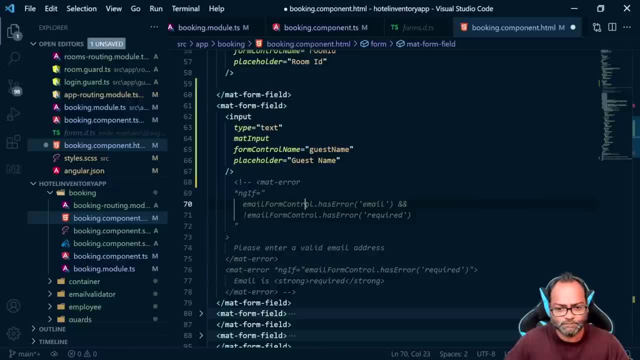 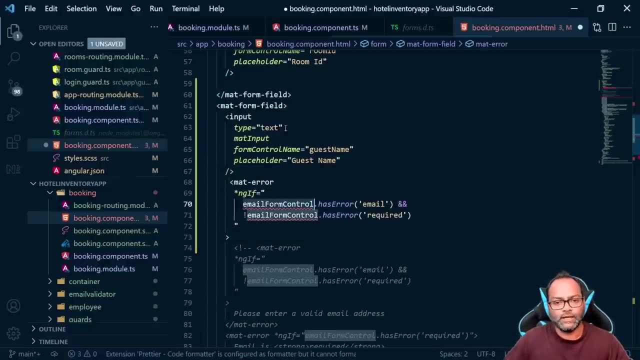 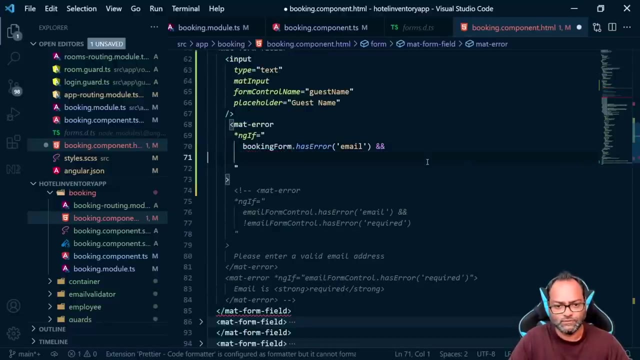 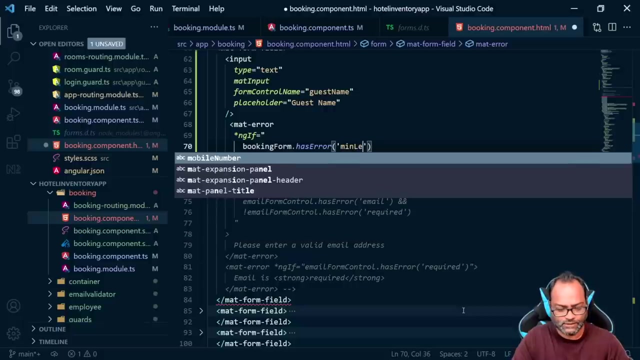 five characters and how. the way you can do it is: let's copy this. so it has a API. so this booking form has an API where you can check has error method. so here, let me just remove this, because we just needed one validation, we don't need both. and has error which is min length. 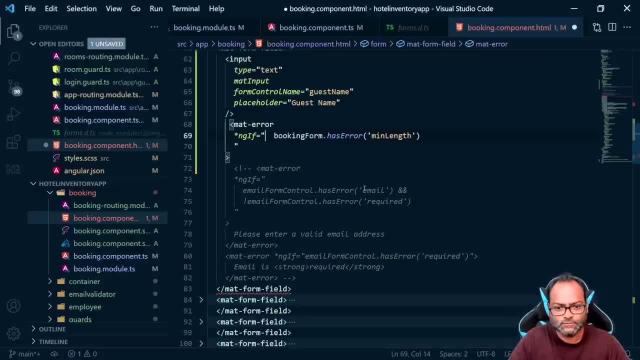 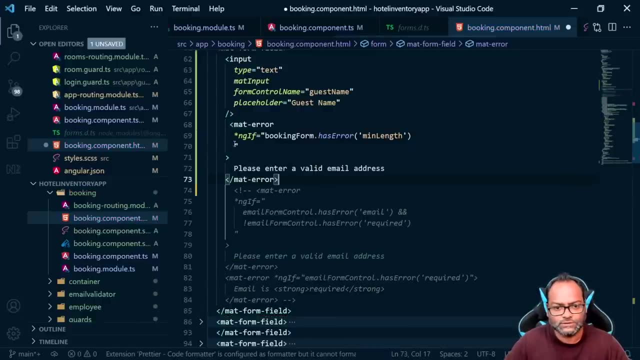 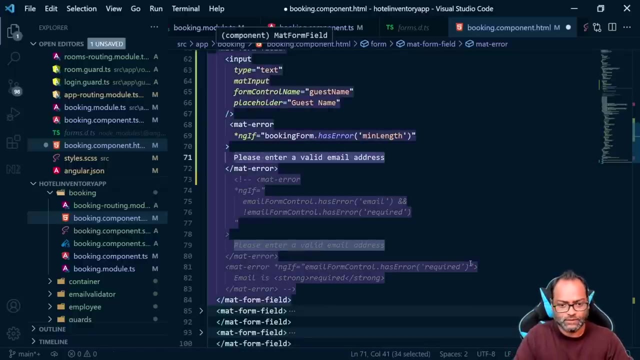 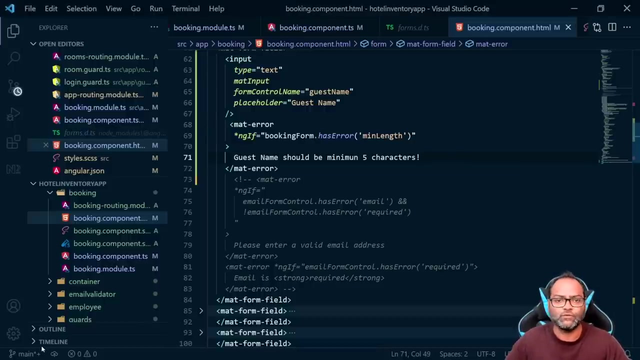 let's format and we can let our users know that. okay, in case it has a min length error, we can say: please, guest name should be five characters, should be minimum five characters, right? so let's go ahead and test this and then we'll add few more validation. 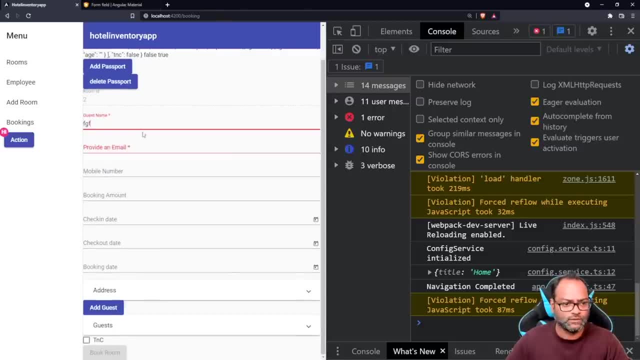 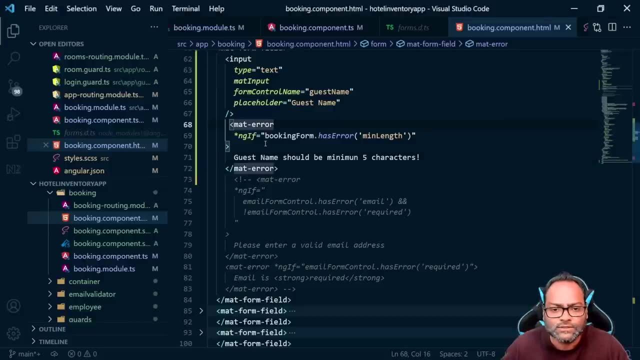 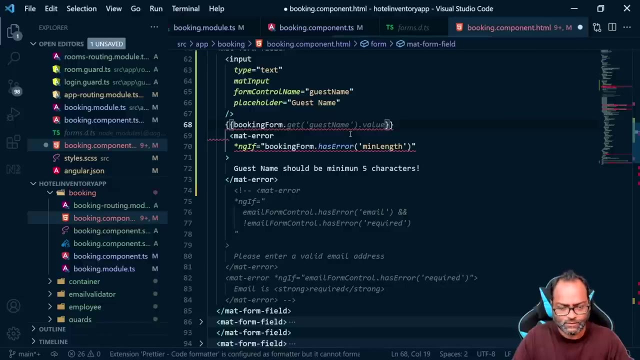 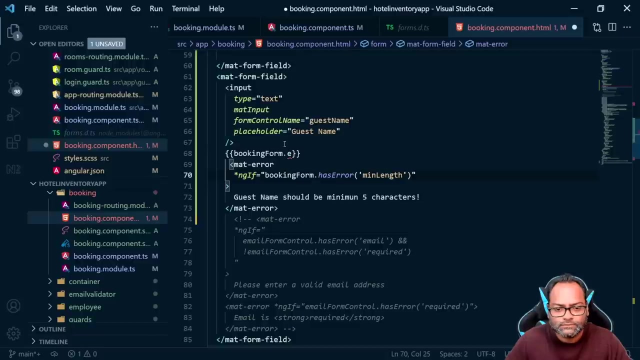 and so let's see, okay, somehow it's not available, let's. is that not saved? let's see now, probably it has to do with booking form dot errors and let's get more information from site so you can see here: uh, we are actually looking at the booking form, which is not 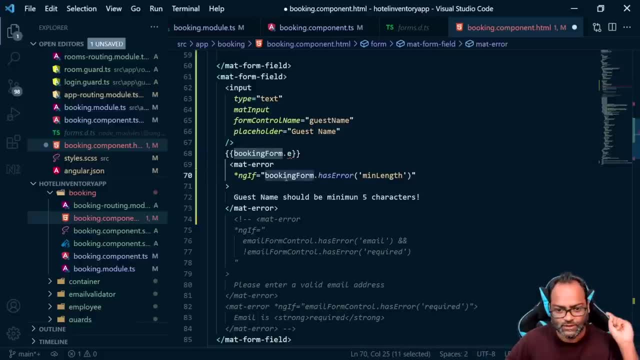 true, because this min length is available with this particular control. and let's see we can, how we can do that. so you, we can do something like this. so, uh, booking form, dot get, and you have to say, uh, the control name, uh, so, which is get. you can add just like this: uh, we are going to get. 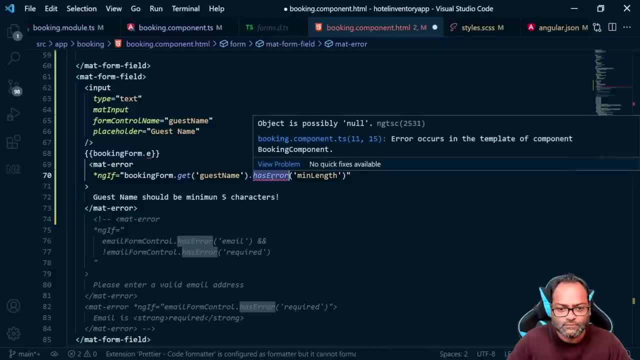 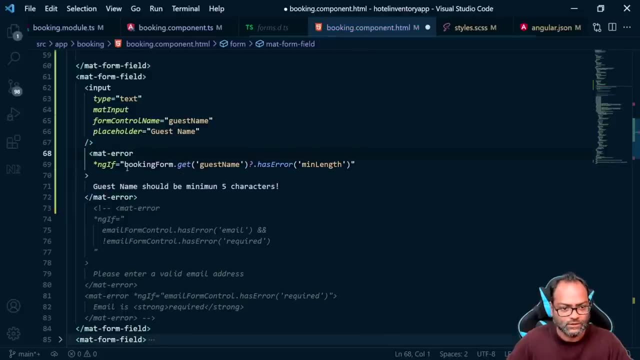 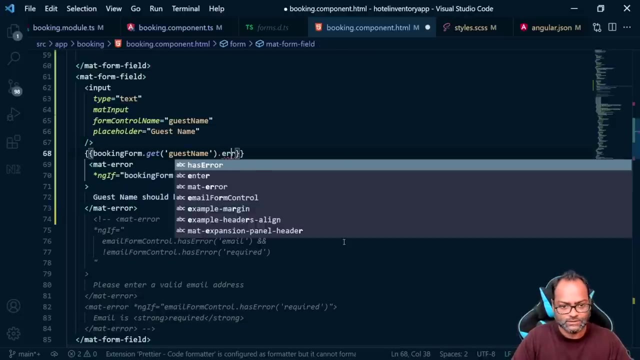 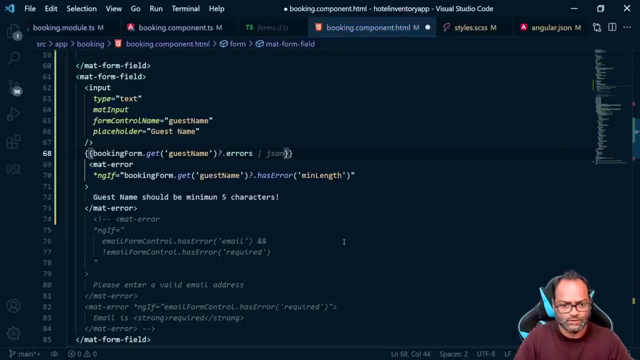 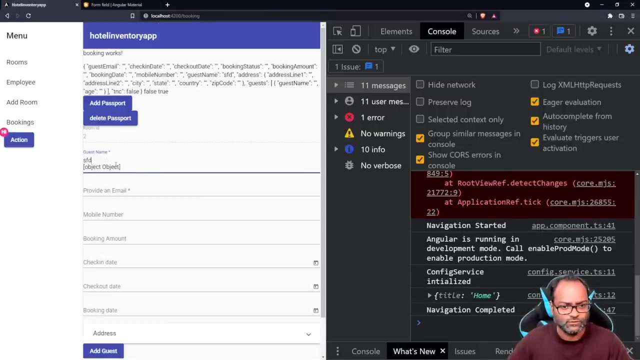 guess name and then we can use: has error, so we will use, as it can be null, let's see. all right, so we can actually do something like: let's print this: dot errors, let's put question mark, so in case it's not null and that's it, let's see. so it says object: object: right now. 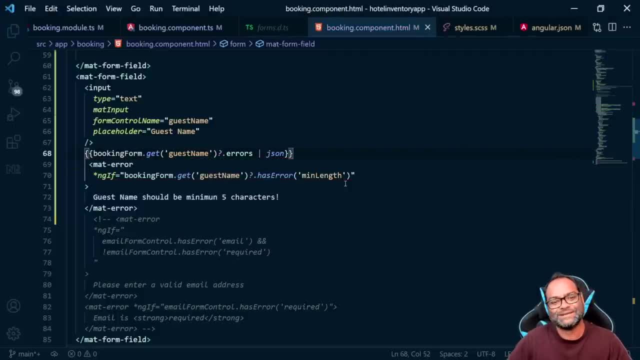 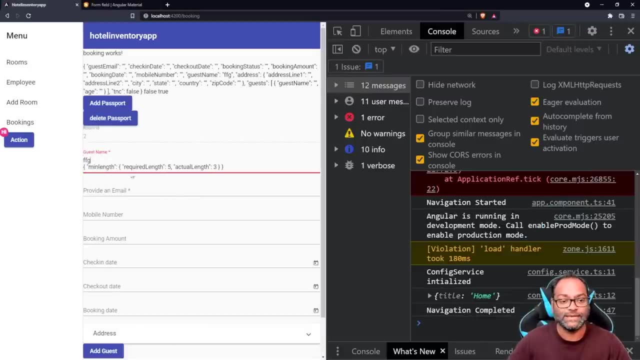 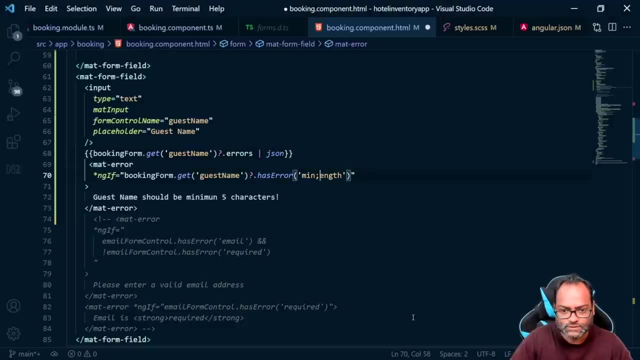 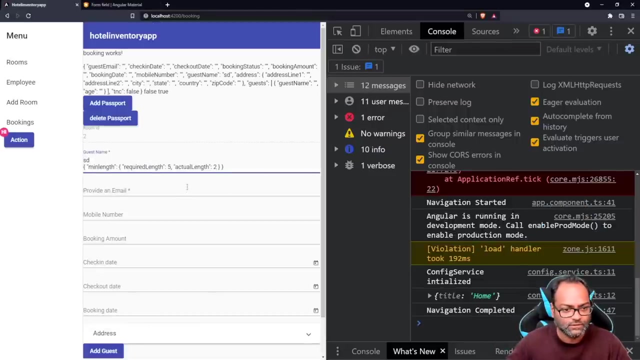 and the reason being: it's actually an object. so let's see, we'll just do json because it's right now required. true, and you can see now it has mill length error. so m i l l l small and we should now have this error message. you can see, guest name should be minimum five characters so we are able to display. 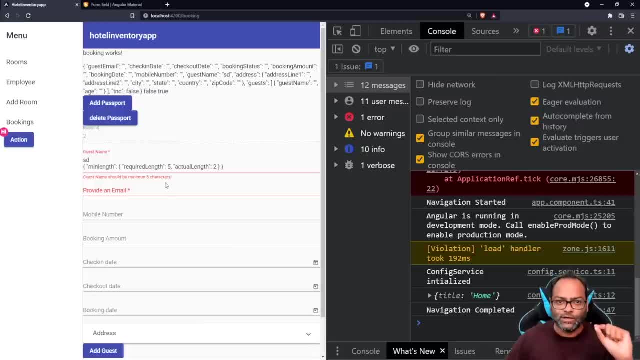 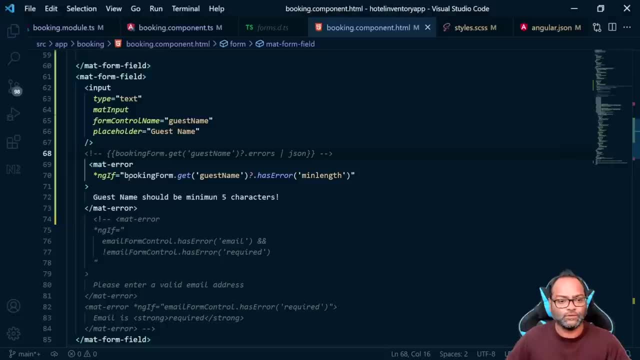 the error based on your current control. remember this. so, uh, we'll remove this one, comment this one so you can what you can do. you can just so use a booking form to get the control and then use hazard method to and check if it has this error. 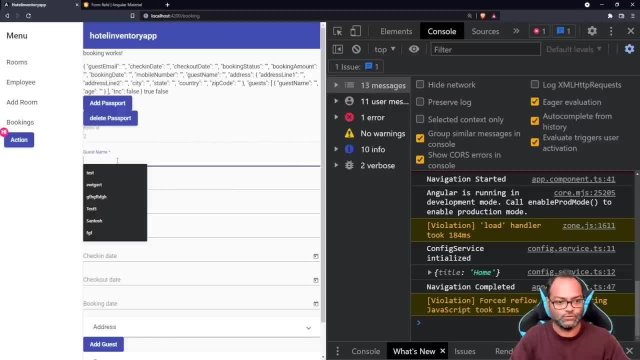 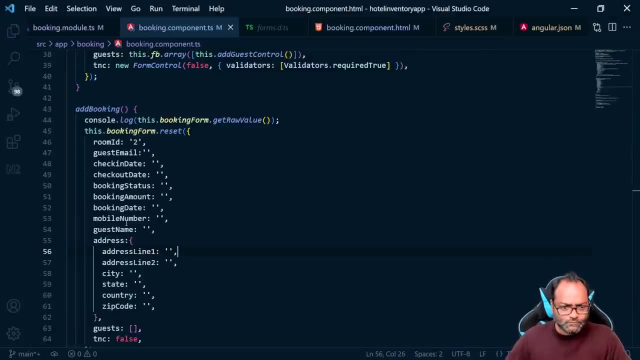 specific error and that's it. that's what you need to do. so now, uh, if i try to move and if i enter less than five characters, i know the exact error: that, okay, guest name should be minimum five characters, so i have to enter one more character. now you might be wondering: okay, this is okay. i mean this. 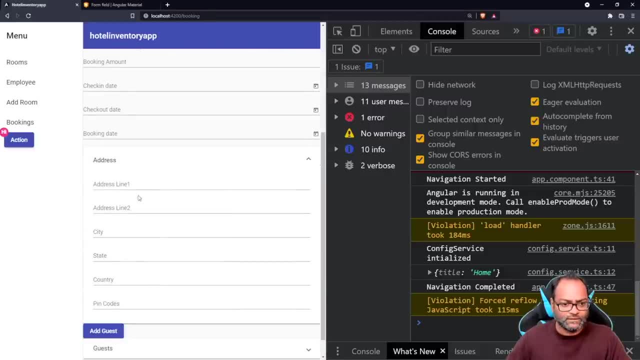 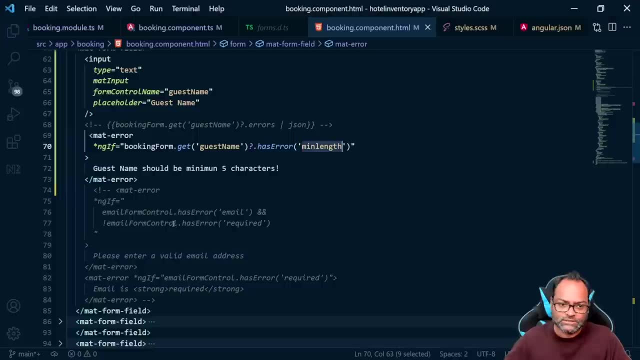 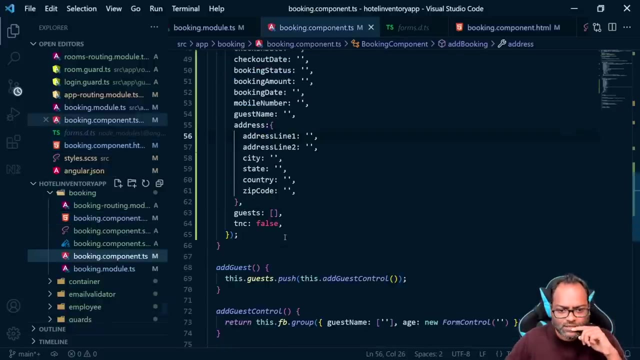 is my top level control. what in case, i want to validate this address line when it is line two, how to mention? uh, the errors based on the control. so let's go ahead and do that as well, and we will do it for errors. so here let's first add the validation. 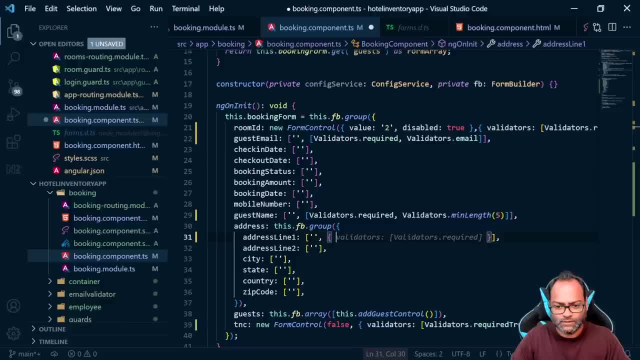 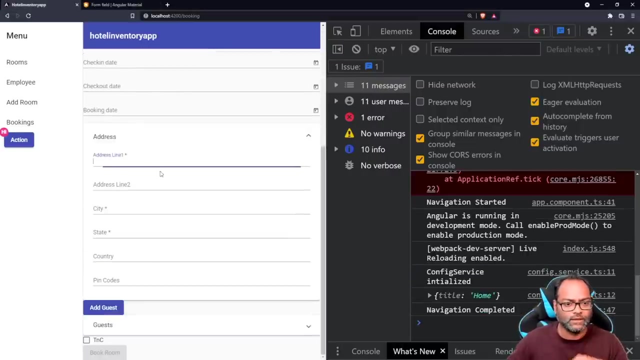 so we will add validators required and let's add it to few more controls. so we have city and let's add it to state. so three, uh, few more controls which are required now and you can see, okay, the validation is already applied. so that's not an issue. now let's go back. 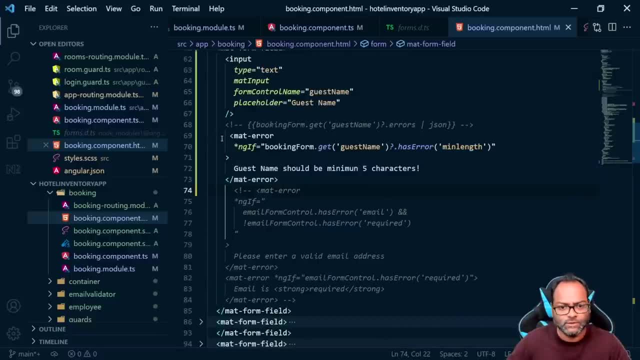 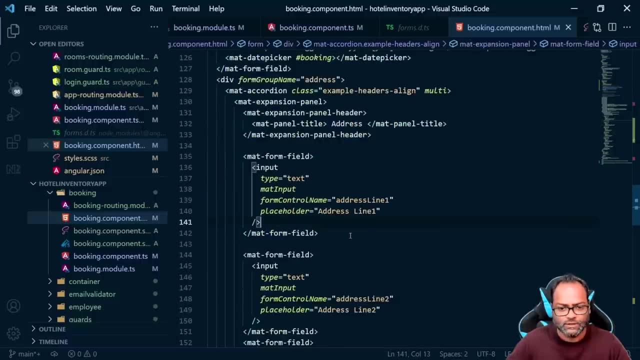 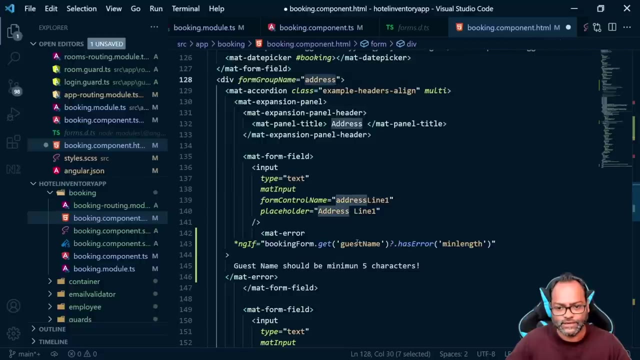 and see how we can show that error. so we'll be using matter and let's go to the address. so address setters, line one here. uh, we will add matter here and we will say: now you have a to actually combine this. So you have to say address get, address dot. 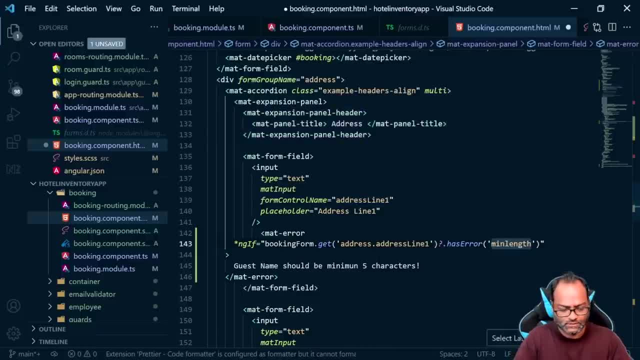 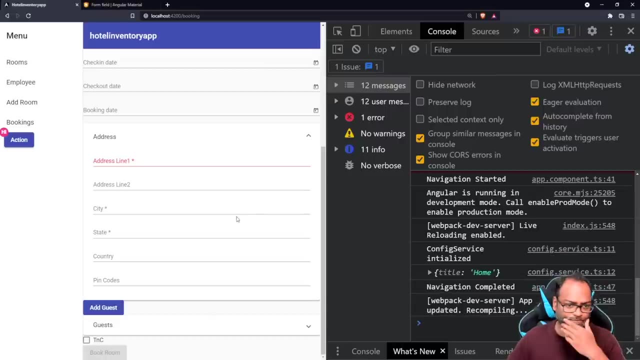 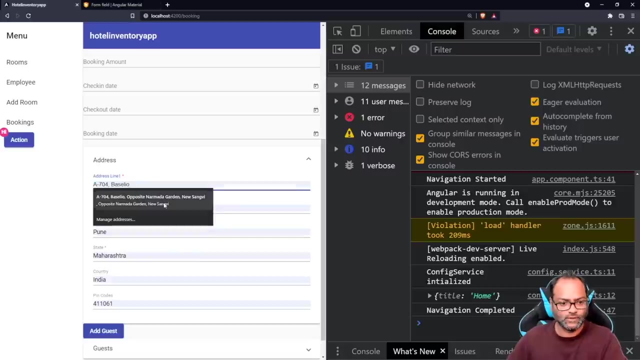 address line one and has error. let us say required and we can say: address line one, is it quite? let us see? oops, this is my, so you can see it says: so you can see, it says address line one is required, right? So we just added this. 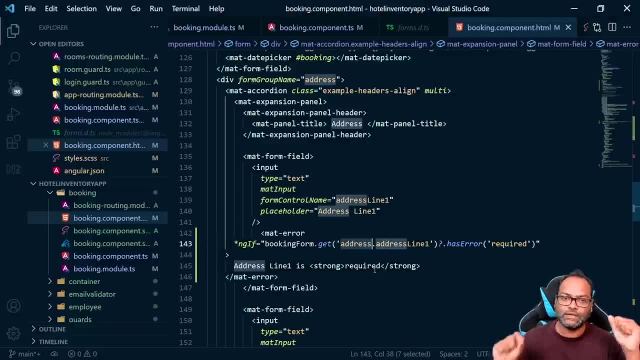 this validation. So remember, for top level it is booking, whatever form name you have, dot get and the control name for nested form. you have booking form, dot get your form group name, dot your control name and then whatever error you are looking at Now, how about the inner sorry array, right? So 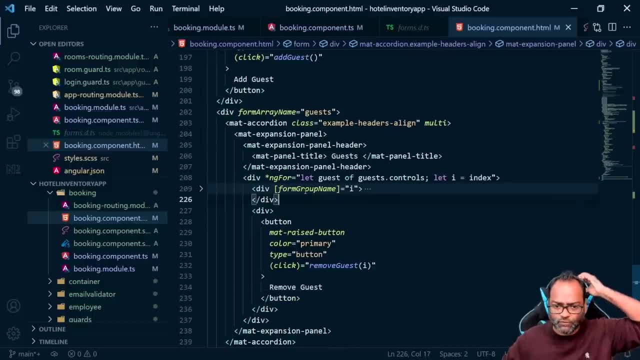 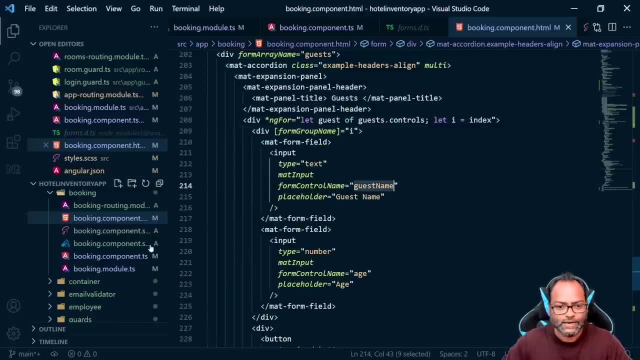 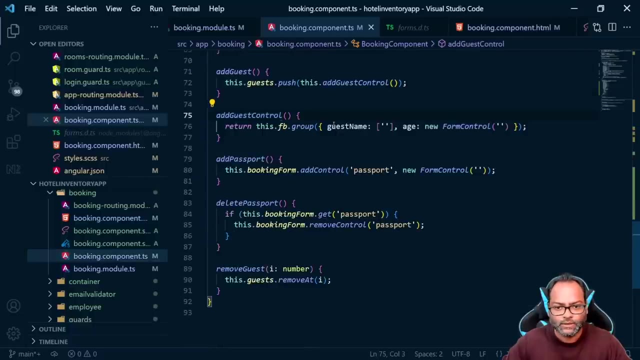 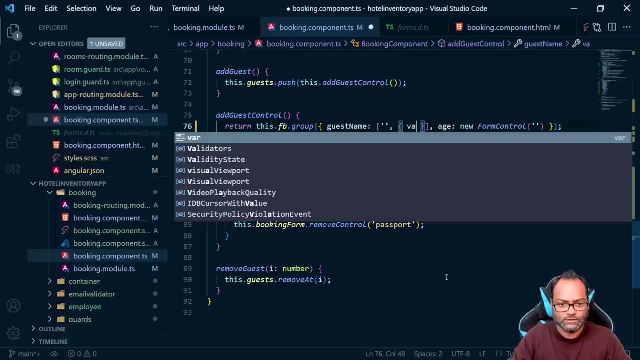 for array. now we do have your form group name, but we also have form array name. So let us see what we are going to do here. So we will add for guest name. let us go ahead and add this guest name and we will say: this is value daters. 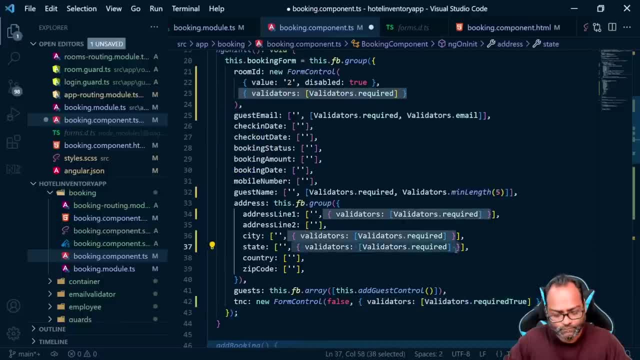 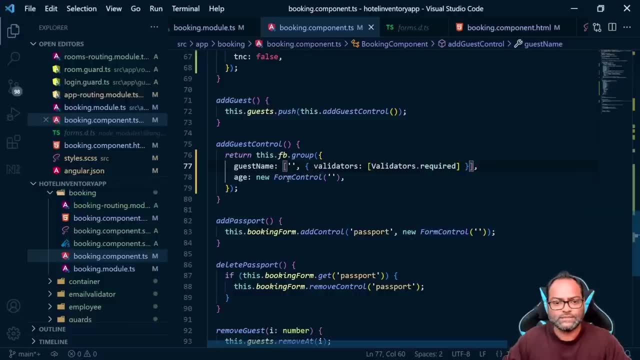 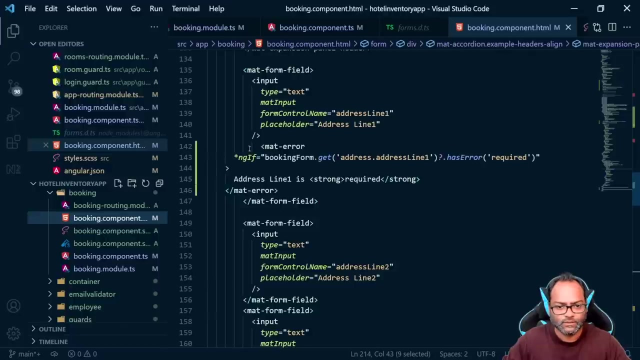 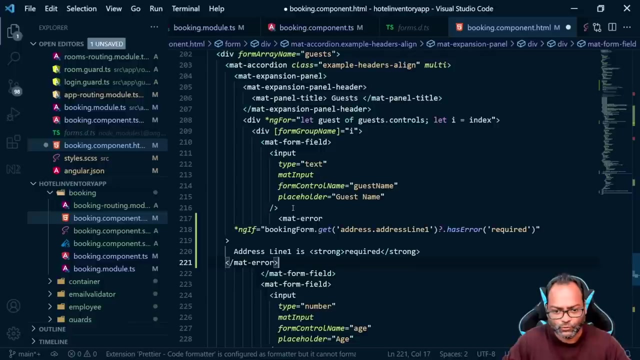 yes, so we have this guest guest name as required and let us see if it is required. and yes, it is required, now let us go ahead and add the validation. so here uv can let us copy this matter thing again. matter come back inside form and this is mat form field where we want to add this error. So here, now it 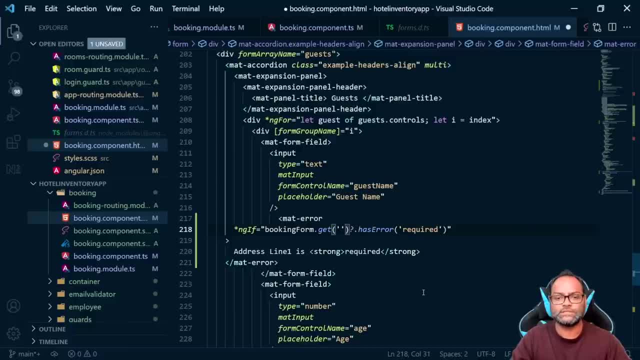 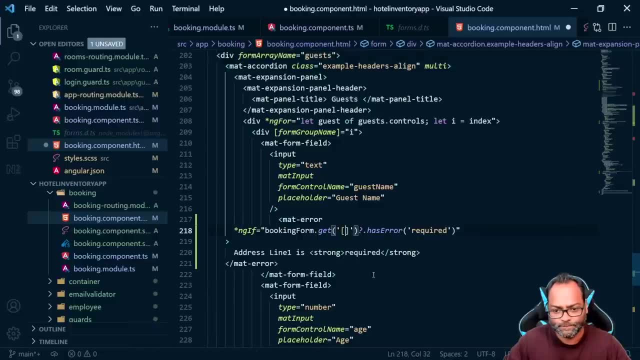 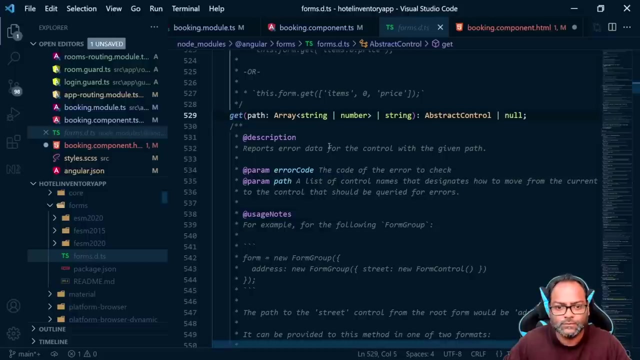 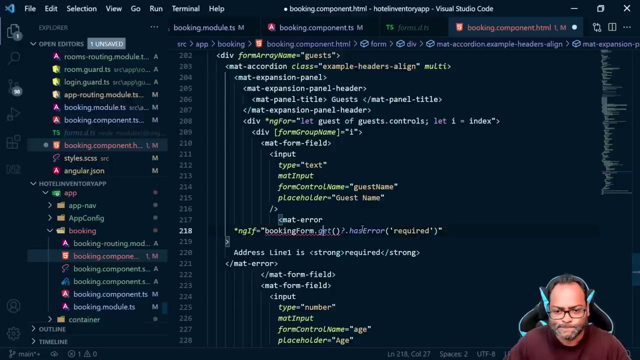 will be little bit different. so now, so now. so now this is an array, so the thing is you have to pass it something to pass it like this. so first is your form array, name comma, so path for array. it's first is your guests, so this will be string, then form group name, which is i. 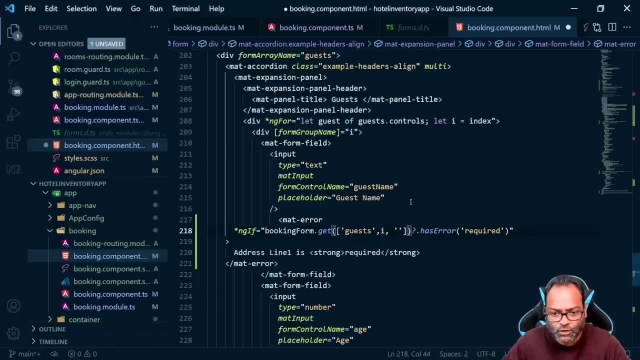 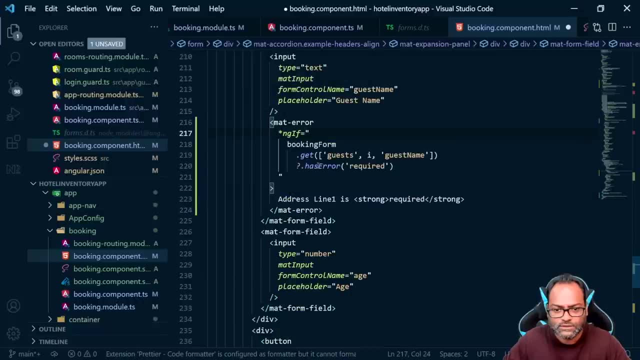 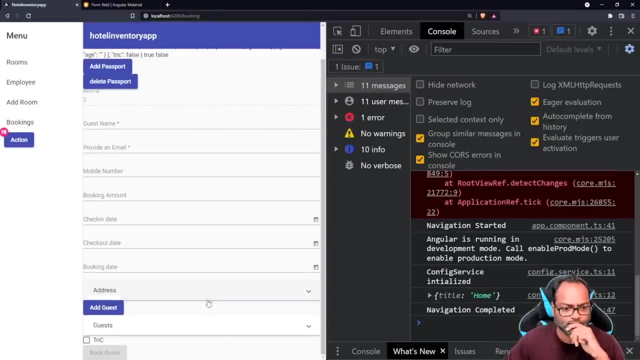 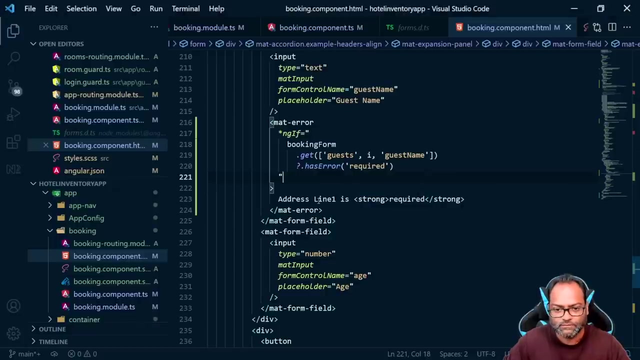 and the third one will be your control. so which is guest name, which is again string? let's format this so we have guests, i and guest name and then has required: let's see go to guests and you can see. right now, of course, we just copied the same so we can say: 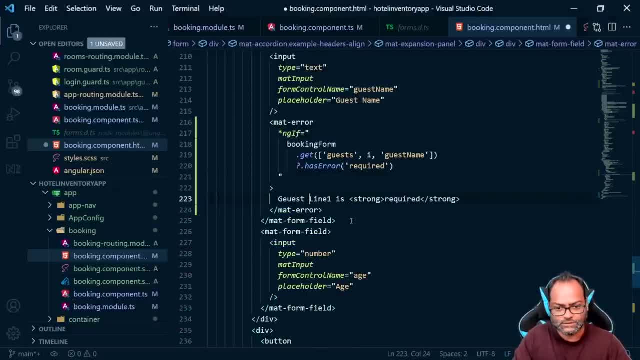 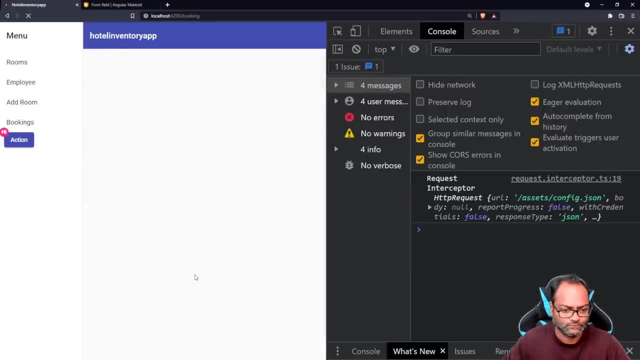 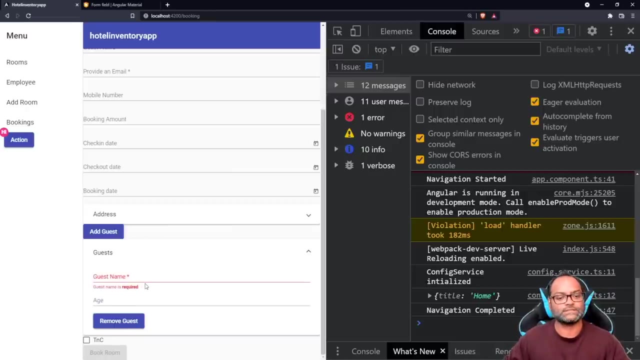 guest name is required and let's try to enter, delete it and move on and you can see the guest name is required. so this is how you can actually display the control level validation based on the target you have set. so you can see the target is set. so you can see the target is. 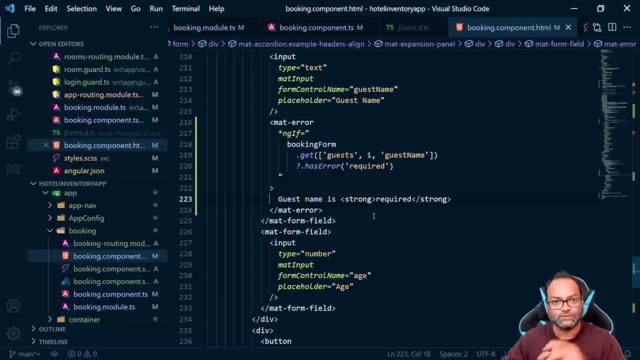 on what field you are trying to validate. so we started with the top level controls, then we went to the nested form and then finally we went to the array. so this is from the. this is it from the validation part, because the sorry built-in validation part. so we learned about how you can. 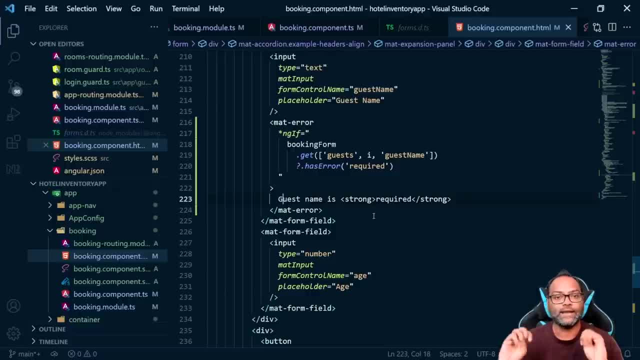 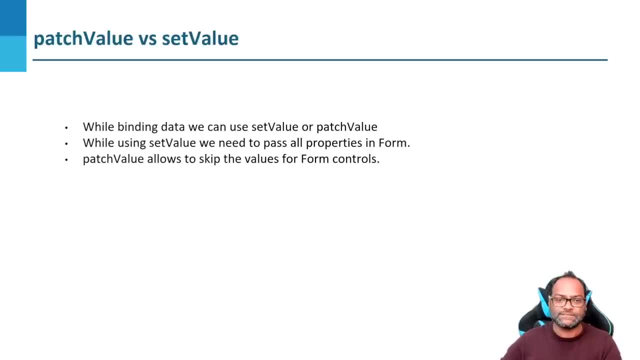 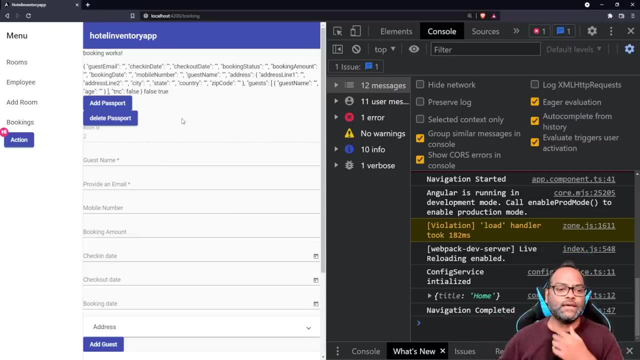 reset your form and how you can go ahead and add the control level validation. we are going to talk about two important apis, which is available with angular reactive forms, which is known as patch value and set value. so first let's understand where it is useful. so right now we have this form. let's say what in case we have this. 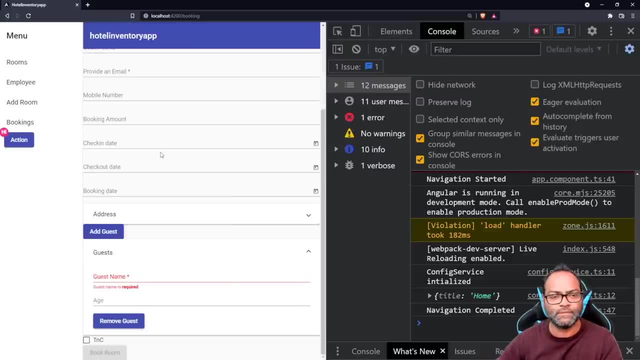 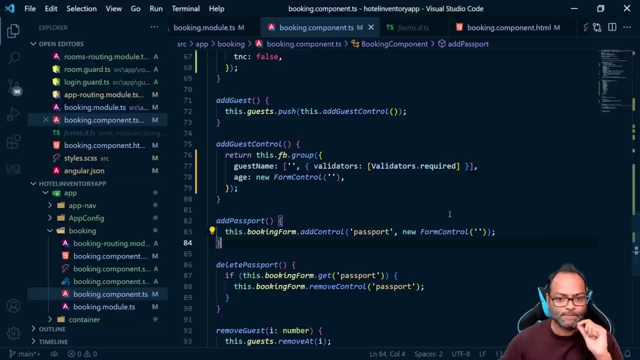 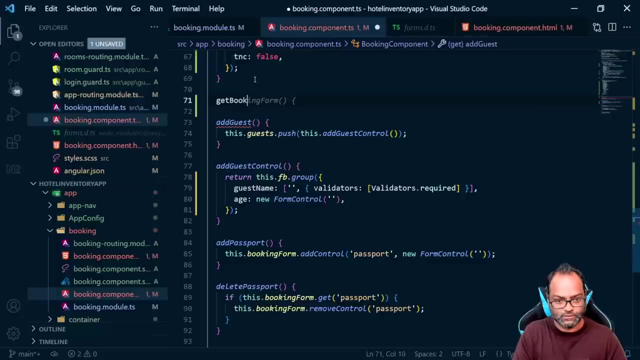 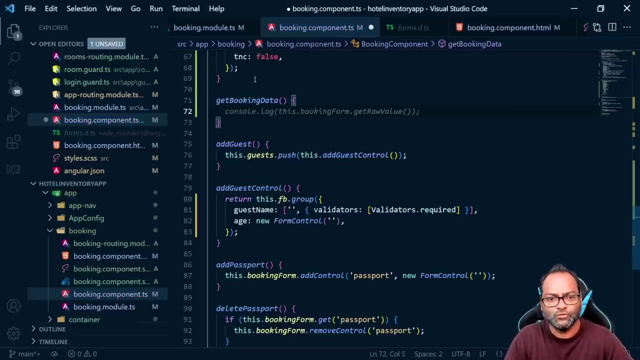 form values coming from some api, how to bind that value here. so let's try to do that first. so let's say we have get looking data. this is a method so we can achieve it in by using two value, two apis. the first is patch and second is set. so i mean first is set and the second is patch. so we'll. 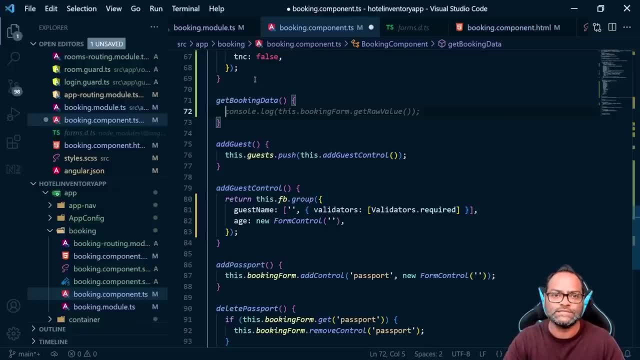 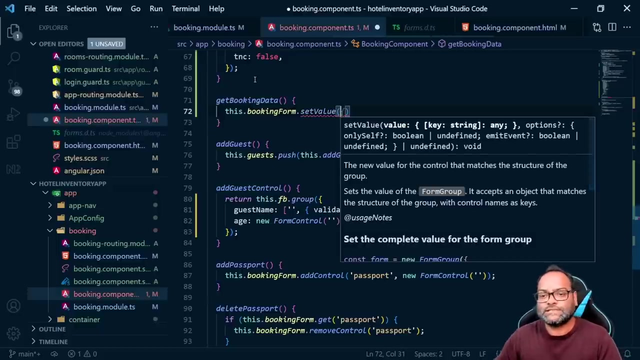 talk about both. so let's see how set behaves, set value, and then we'll see what patch values can do. so here we can use this dot booking form, dot, set value. so this is the api and it takes. so, if you see this the api, so it says values and it says key and value. right, so remember this key. so key is the form control. 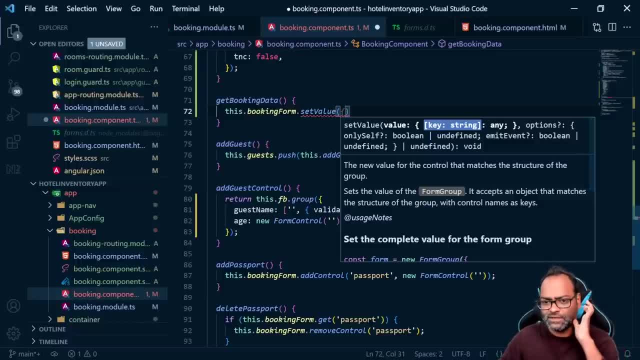 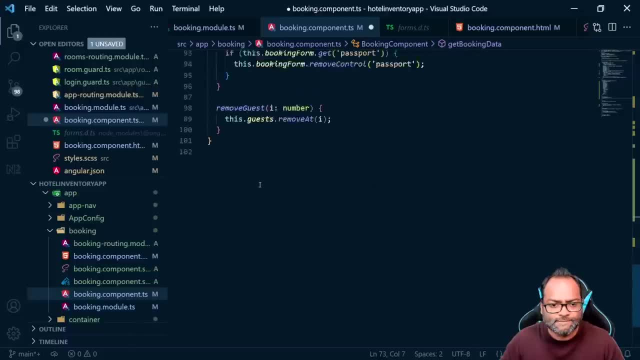 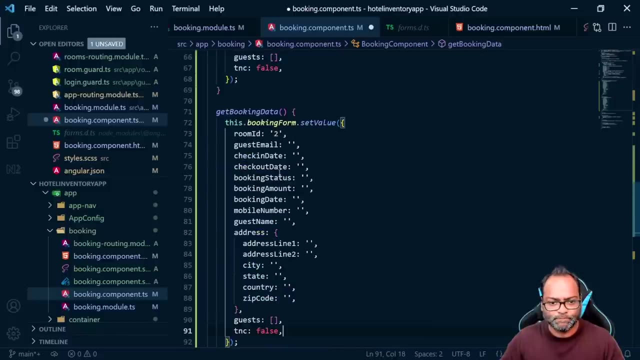 name which we have, and then this is values, and then you can pass some other values which we'll see, which we don't want to see right now, but yeah, so here you can pass the default values. let's say it's coming from back end, right? so? 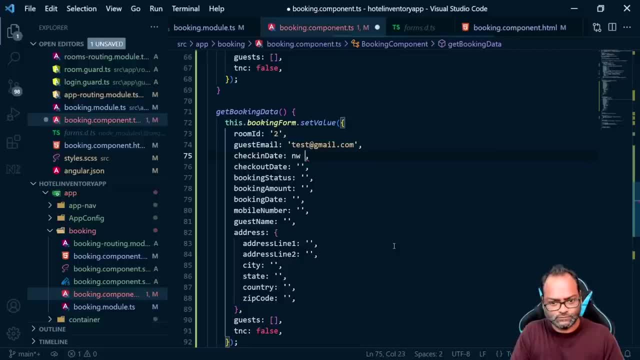 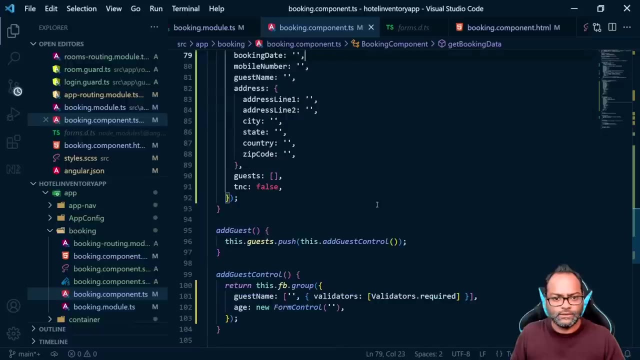 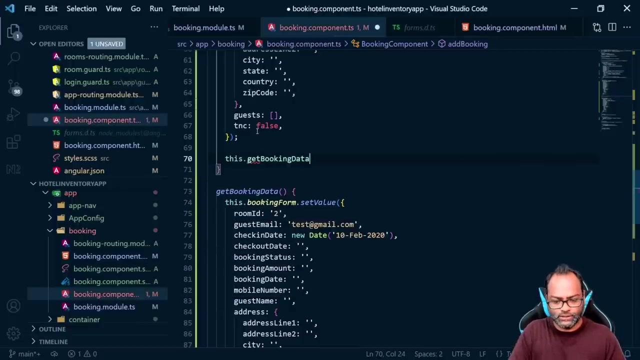 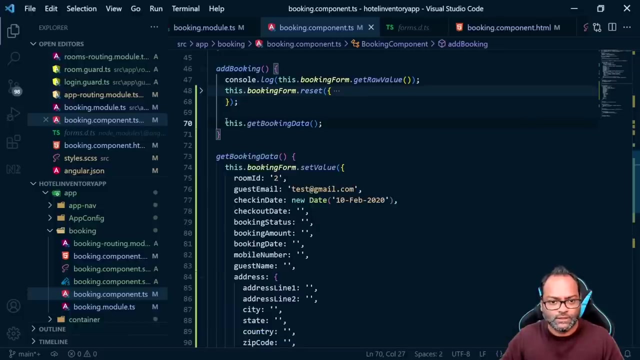 you can date right now, it will fail. but let's see, and let's call this after our form is created. so this is where we will call this the start. get booking data inside ng on it, remember. so i'm just calling it after our. okay, sorry, wrong place. 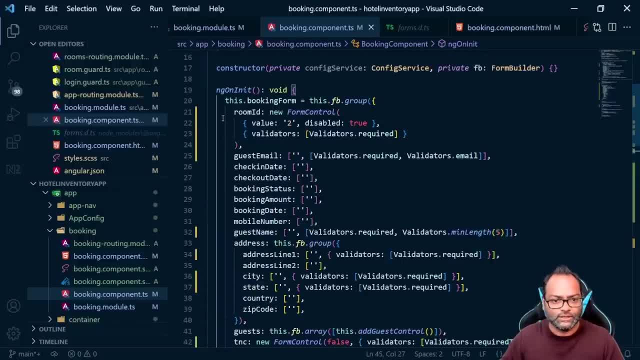 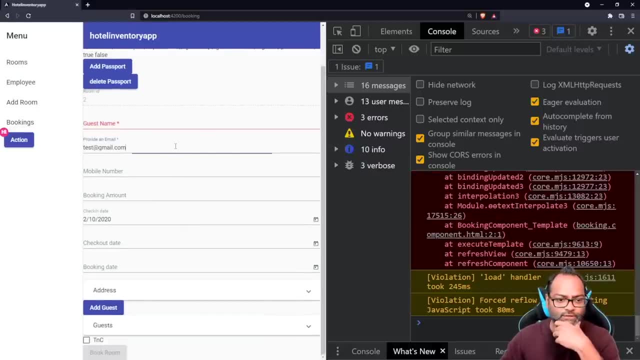 so we need to call it after our form is created inside ng on in it. so here our form is created and then we are calling get booking data. now let's cut and see. so we have all these default values right available here because we provided all the 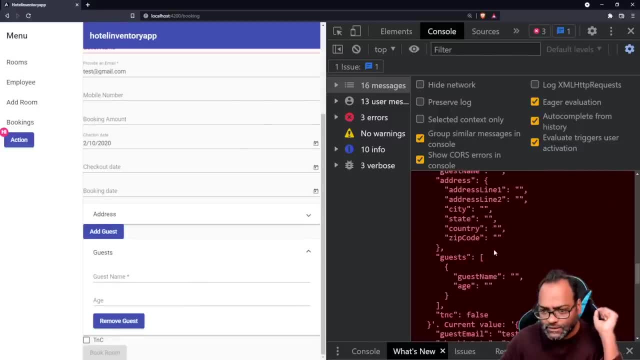 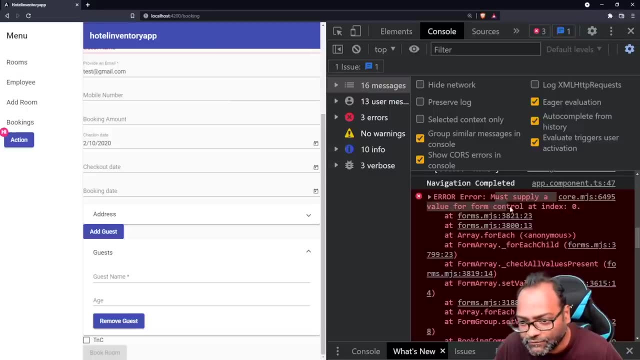 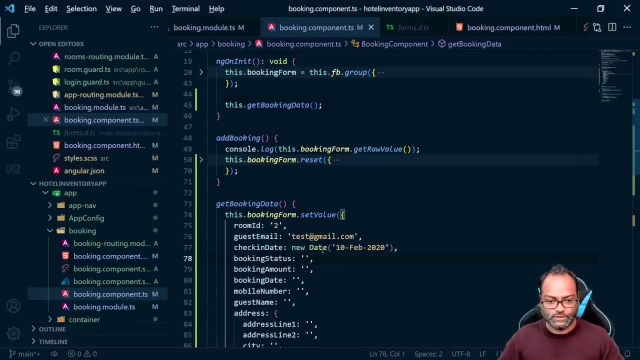 values. but here you see, yeah, that's fine, we don't have uh, yeah, we have an error here, so must apply a value for form control at index 0. this is what i wanted to show you, uh. but let me just do one thing, let me just remove any of the property. see this error. must supply a value for control with name. 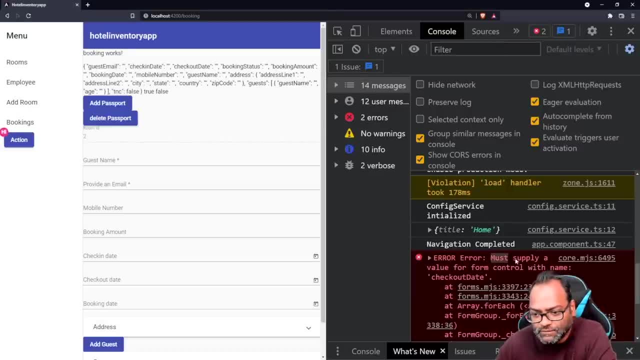 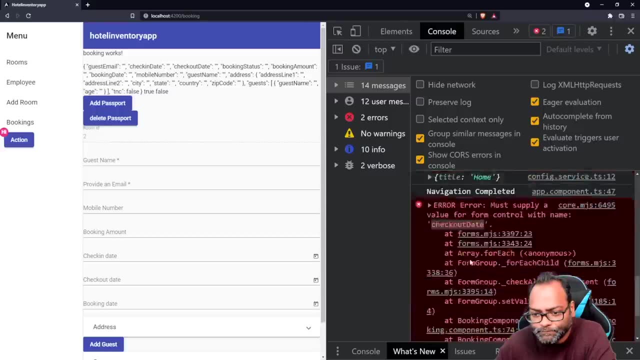 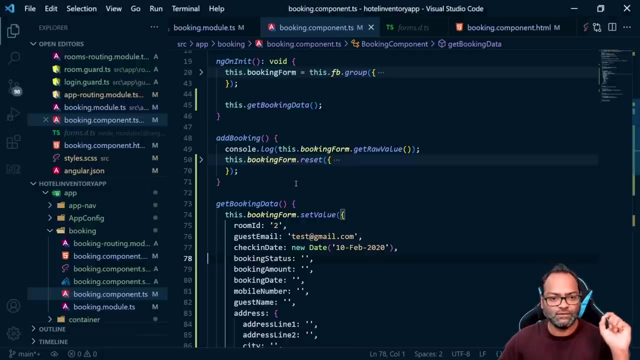 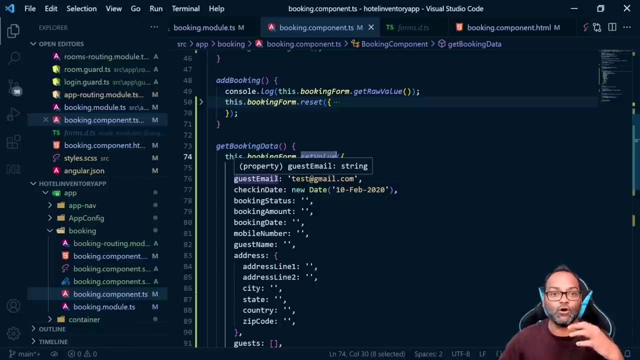 checkout date- and let me just remove any of the property. see this error- must supply a value for control with name checkout date. and why so? the thing is, whenever we use set value property or set a value api, it expects us to pass all the values for all the control which 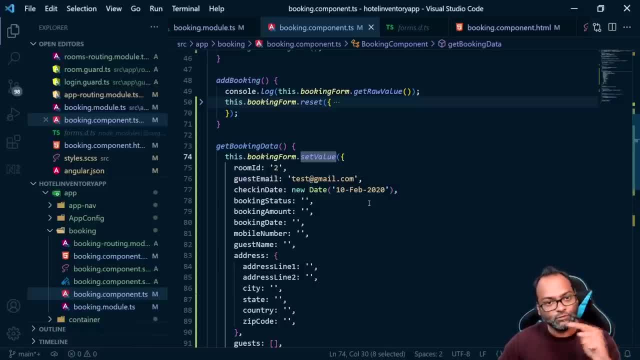 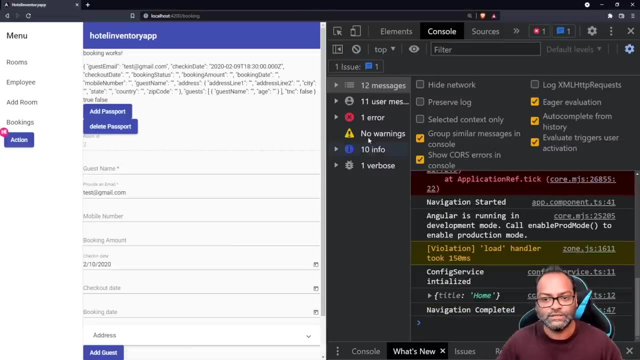 it has. keep this in mind. set value. we need to pass the value for each and every control, patch value. it makes it a little bit loose, so in patch value you can- you are allowed- to skip some of the controls. so now you can see we don't have the error anymore and everything works right. so if i 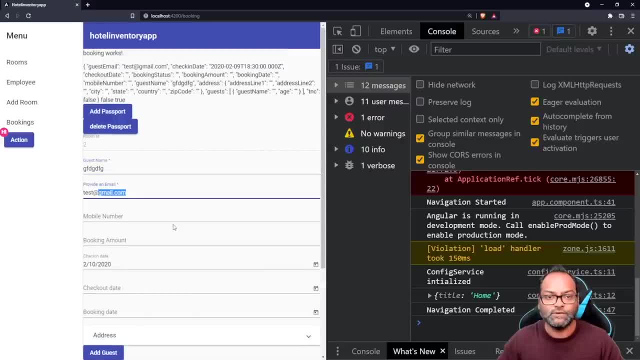 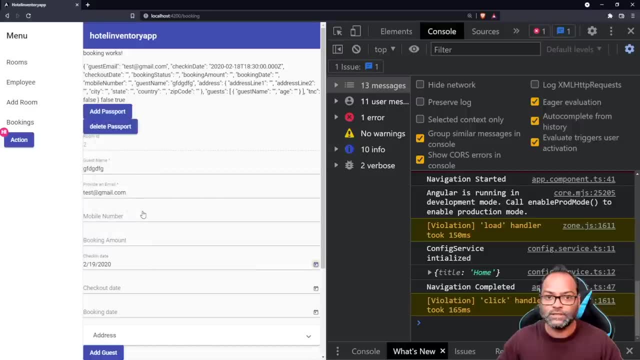 just provide guest name, it will work, and we already have this value, which is provided or set using the patch value method. so this is the difference. otherwise, there is no difference between set value and patch value. set value makes a little bit strict that you, you have to go ahead and pass. 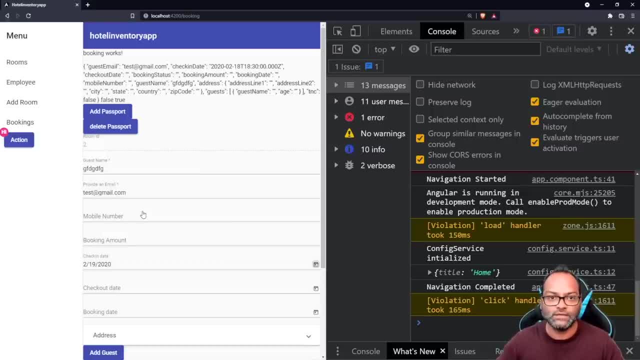 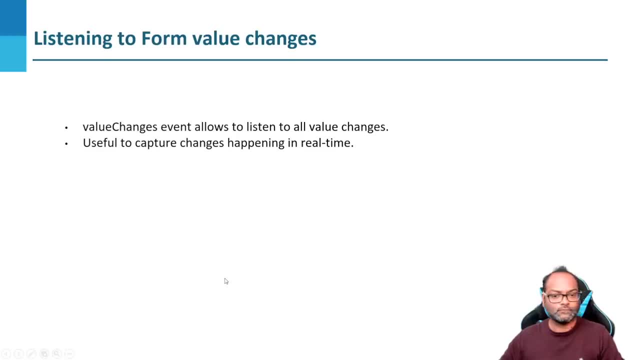 every value for each and every control. patch value makes it a little bit flexible, so i don't have to pass everything. so i'm just going to use the same thing. so i'm just going to use the same thing. so form api also allows us to listen to the form value changes in real time. so 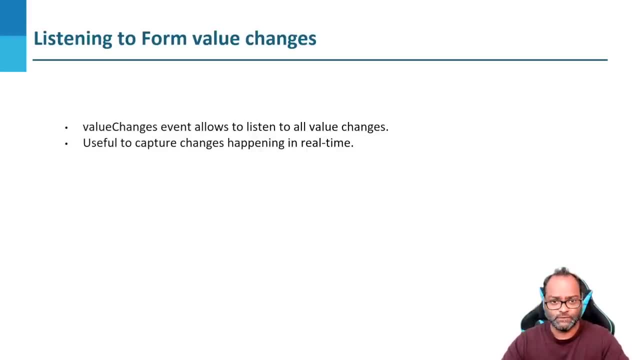 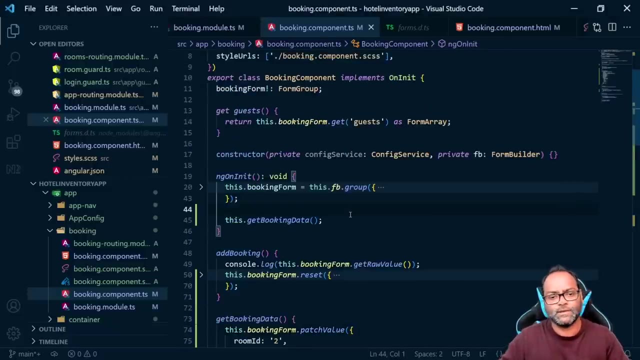 how it is possible, so you can use a value changes property, which is a stream- remember, we have already discussed about stream, so which is a stream and which looks for any changes which is happening in real time on your phone. so let's go ahead and see how we can actually utilize this api. so here after, 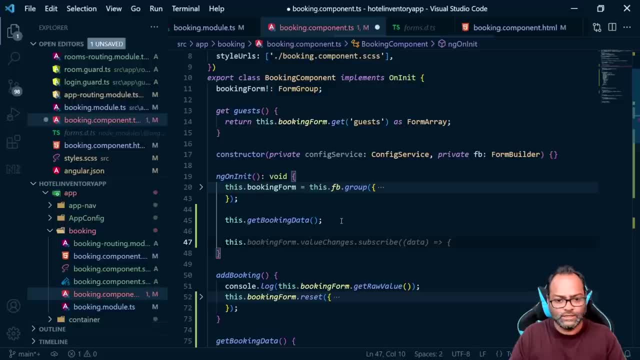 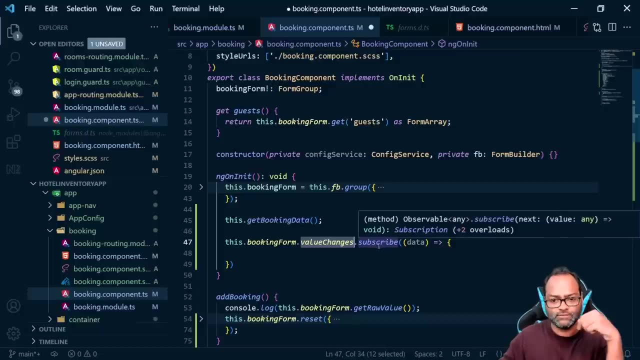 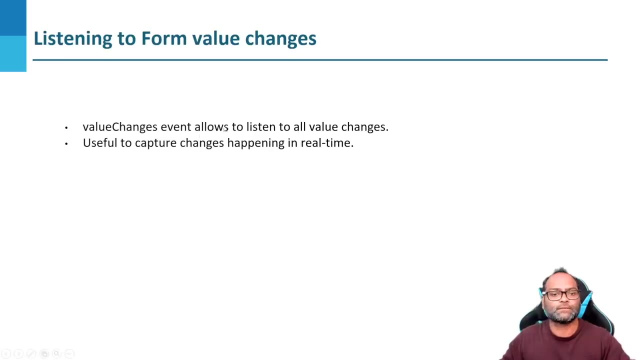 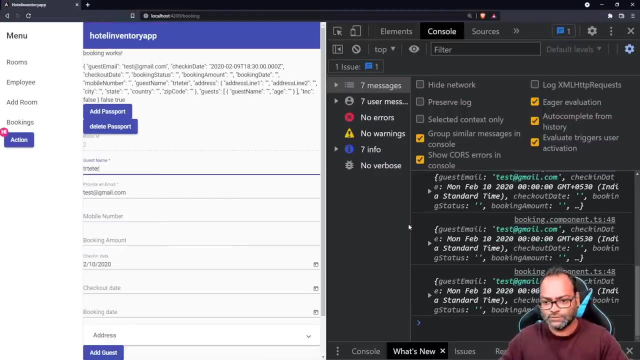 my form is done. we can actually use booking form dot value changes. as this is a stream, we are subscribing to it and it will give us the data in real time. let's see so consolelog data and let's remove this and enter the value. so you can see as soon as i enter a value, it is actually 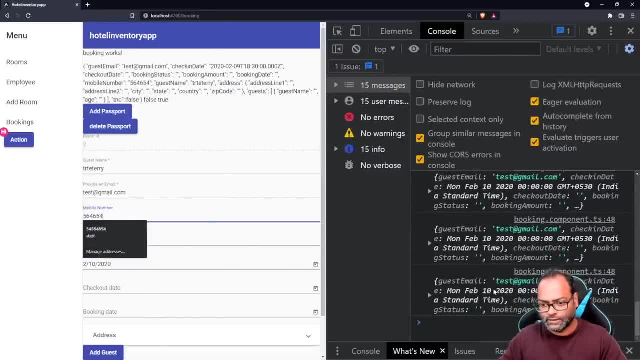 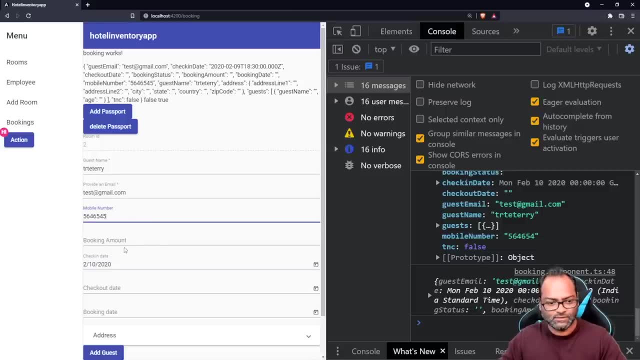 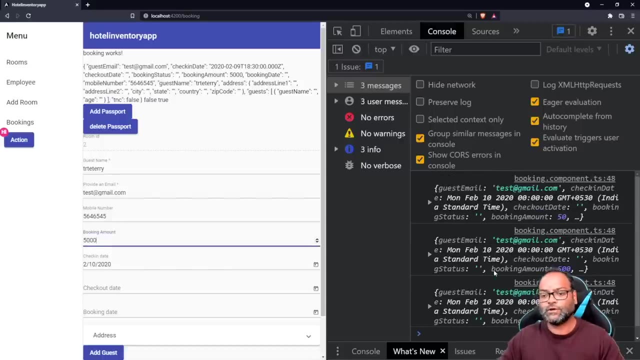 giving me the data mobile numbers, and now we have this mobile number available, so it will be called for each key press, remember? so if i enter five now, let's enter zero, zero, zero, right, so for each and every value which is getting changed, you can capture that value in real time using value changes. but it isn't it an overhead? 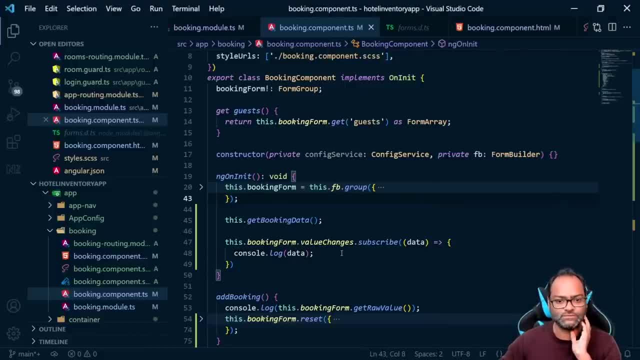 i mean, why should i need to? i need to know the value changes which is happening in real time. but remember it means in case i have an validation- uh or custom validation- it will be triggered for each key press. sometimes it becomes a little bit uh. it can give you performance issues sometime. 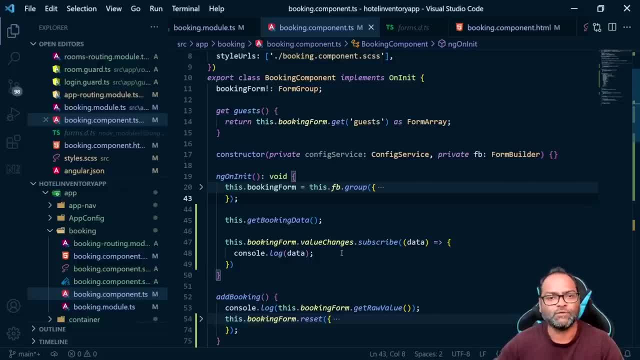 in case you have a small form, doesn't matter. but in case you have a lot of controls and every control has some validation which is getting triggered, it may make your forms a little bit slower. let me tell you, angular is really fast, so probably you will never. 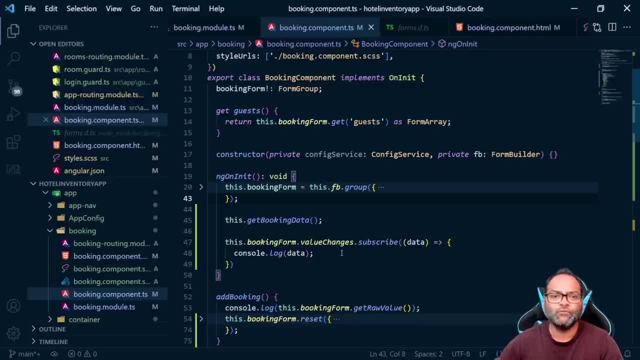 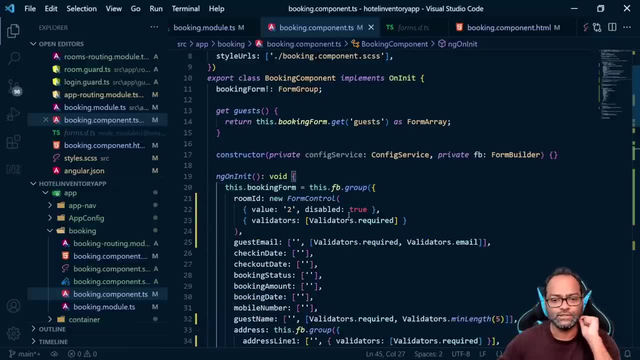 get to see this issue, but just just in case, so how we can avoid it. so let me introduce you to another property which exists on your form controls, which lets you control the behavior, how your form values will be changed. so right now, values get changed on each key press. 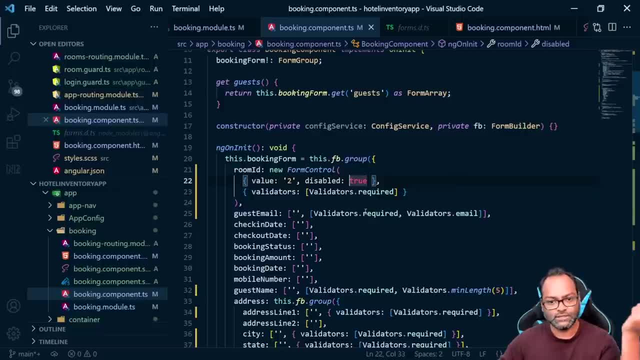 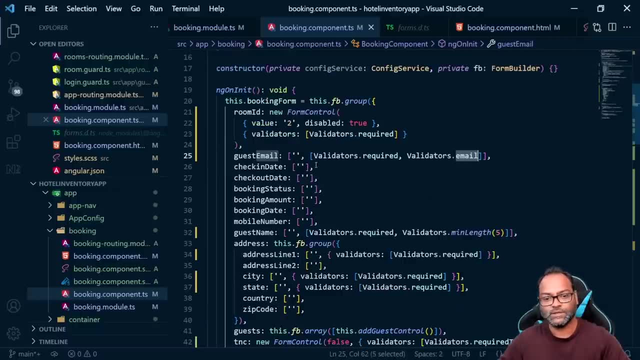 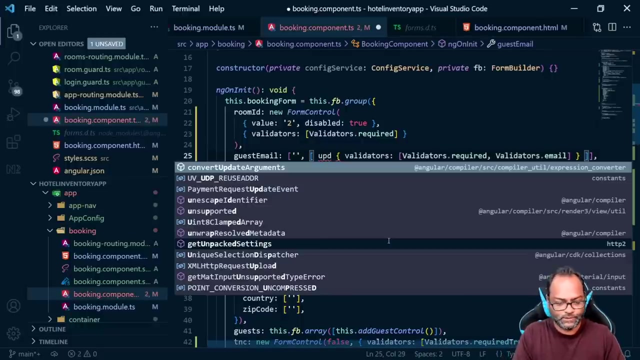 that's a default behavior. to change the current behavior, you can do something like this. so here we have this: validatorsrequired validatorsemail- right, so here we can change this to validators. so we will say: okay, this is a value and there is a property called up dated. 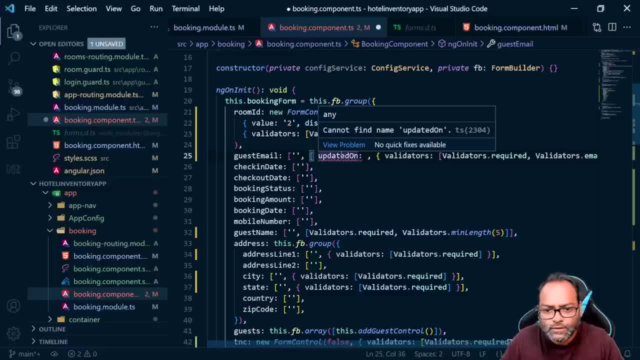 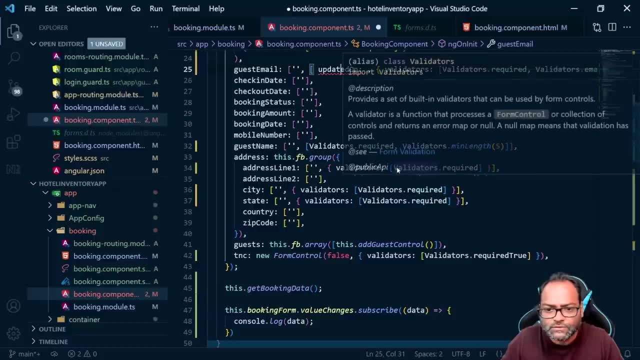 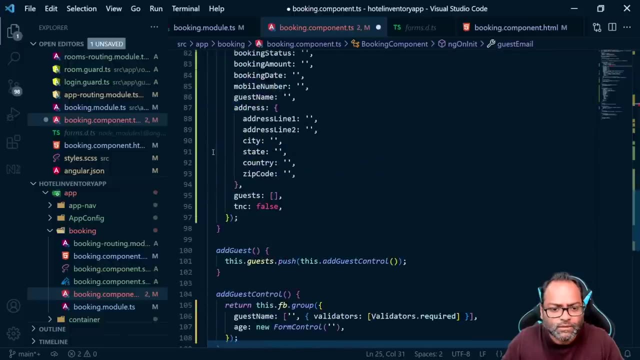 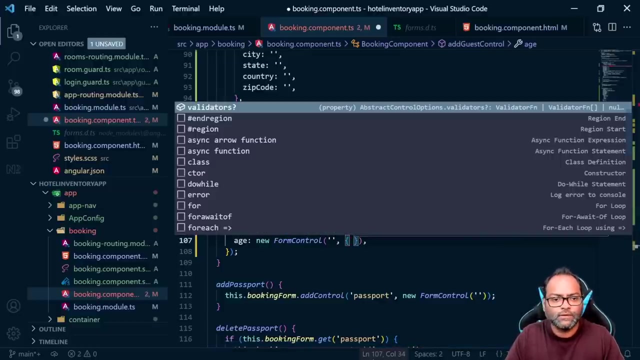 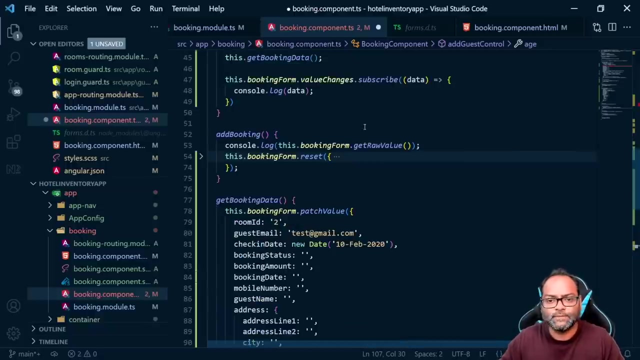 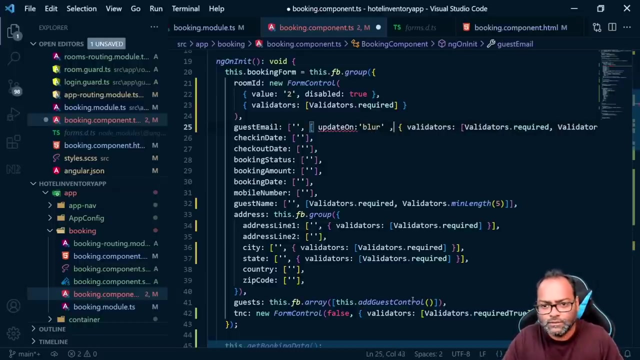 on. that's one second form control. let me say: see where we have used form control so we can add control here. so, uh, we have validators and update on- sorry, not updated on. so update on remove this and we will say update on blur and we need to change this to an object. that's why I prefer 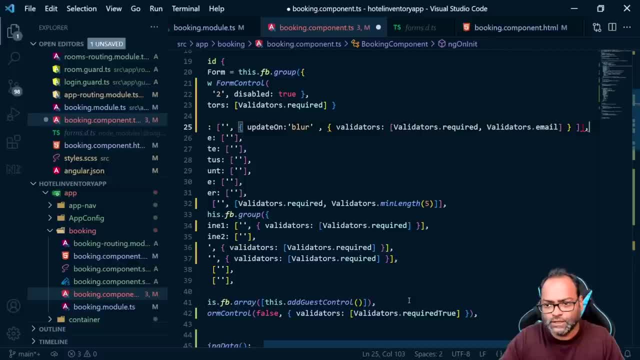 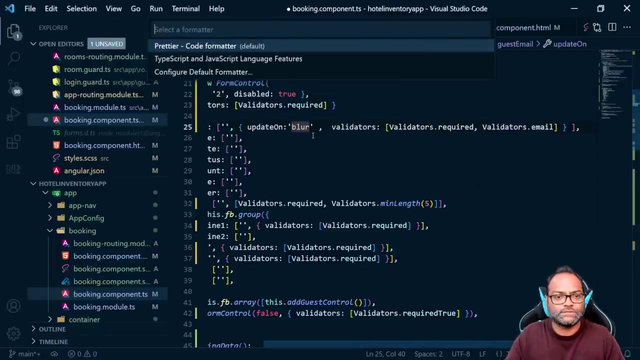 using new form control rather than this. but yeah, it's okay, we will do. update on this is okay, this is okay and this is done and we have an this as an extra. let's see, then we can pass, we can remove this and yeah, let me just format. 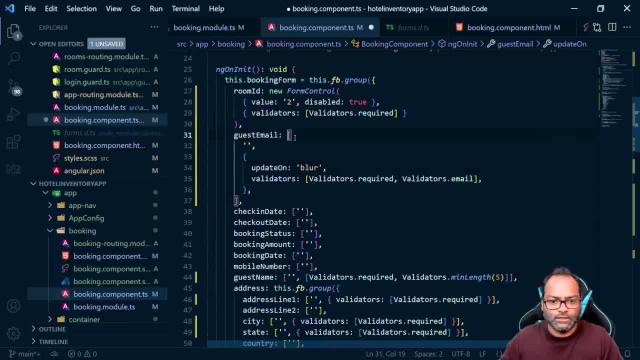 so here, with this, we are passing an object which has two values, update on, and then we have validators. so now for email, and let's add it for some other control as well. let's add it for mobile number, so I can just do something like this. I can. 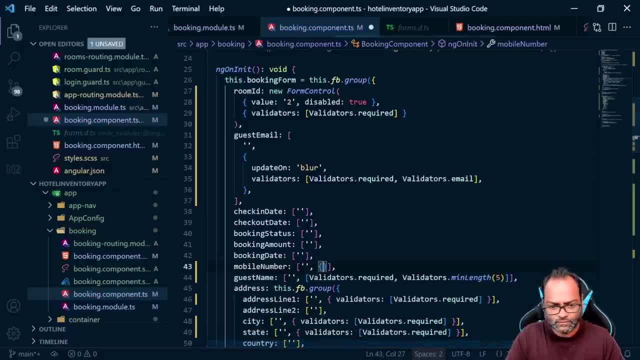 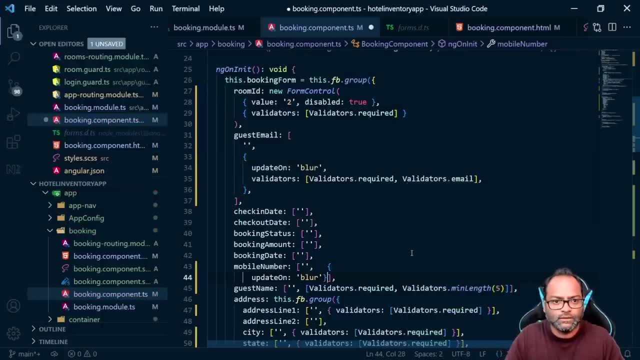 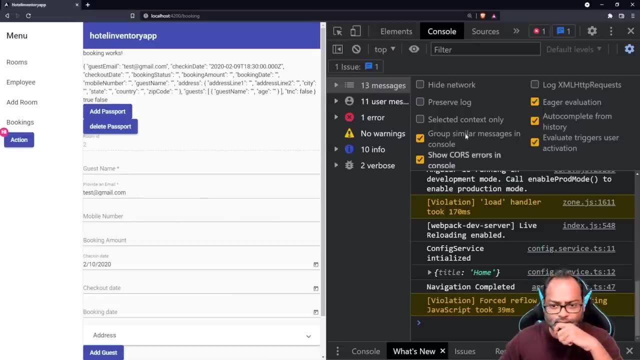 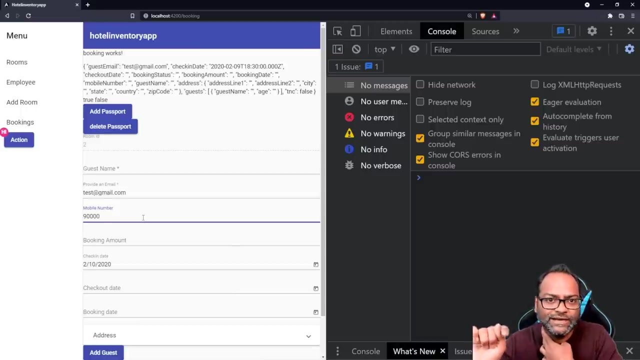 right. so I'm saying this is this will be updated on blur. so blur is an event which will be called once you move out of the control. so let's see, let's remove this, let's enter mobile number so you can see no values is being captured and 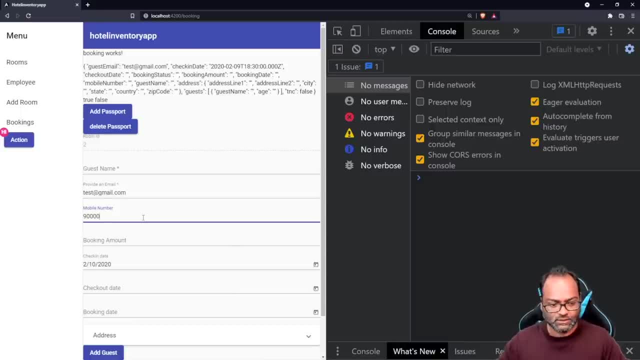 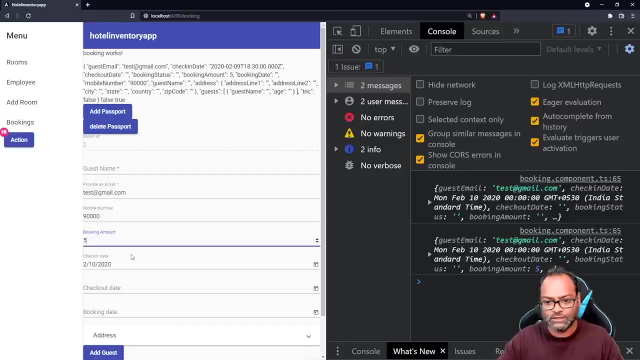 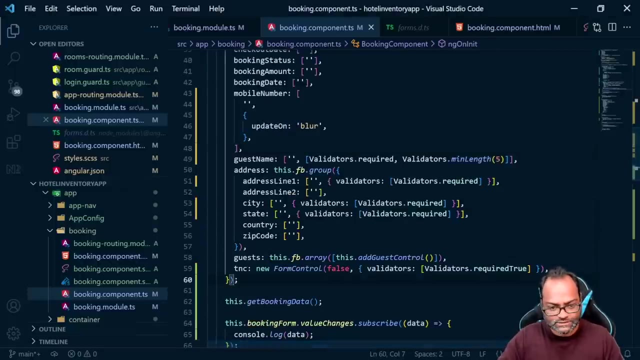 in real time. so as soon as I press the keys, it's not happening. press the tab or move out of this control. you will see the values being changed. for others it will be same. I mean, we have not changed the behavior for entire form. can we do that? yes, we can. you can also pass this value here as the 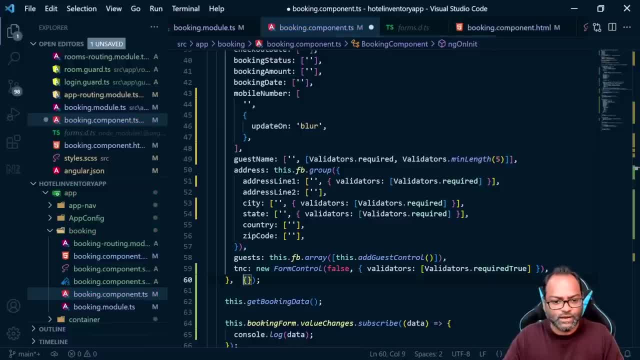 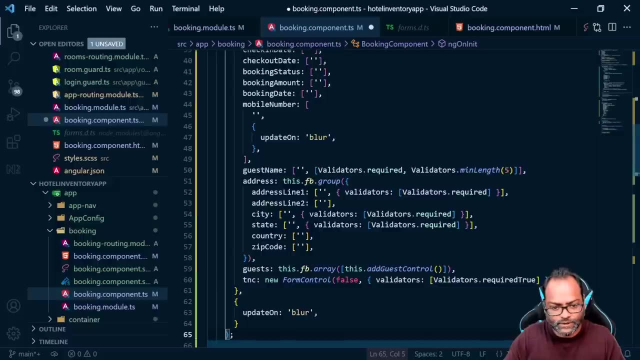 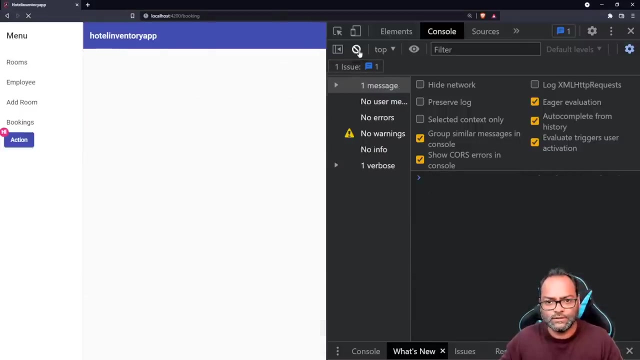 last option, after your form is created and you can pass the same properties, so you can say update, uh, update on blur, and then, in case you have some validations which we will use, you can do that. so let's test it now. let's enter booking amount and you can see it is not getting called as soon as I. 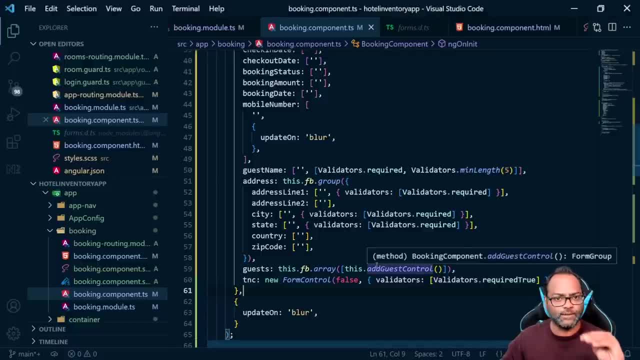 move out of this particular control. it is getting called. so this is the for template driven form. this is how you can be change the behavior: uh based on uh, based on how your user interact. so there are three values which it has. so you have blur change and 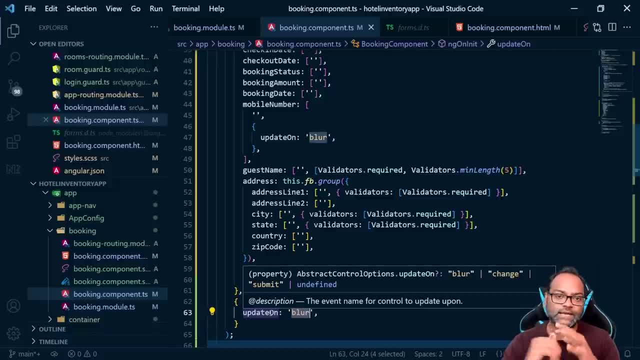 submit changes by default. submit is really useful in case you don't have any errors or any validations, or you want to show the validations once your form is submitted so you can move to submit. so in that case let's try to understand how it impacts, right? so for change, let's say you have 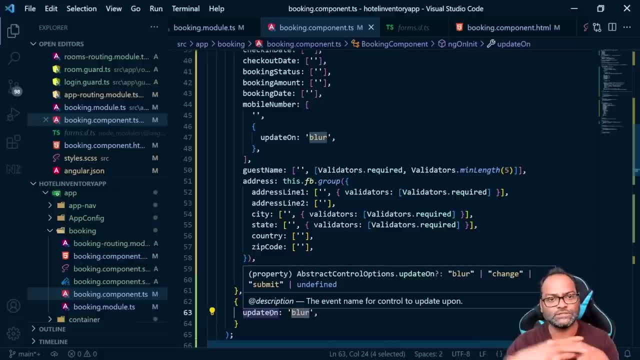 one of 10 controls where I average users enter five keys, so 10 into 5. times your change event will be called in case we move on to blur. it is number of controls, right? so if you have five controls on sorry 10 controls and let it be any any your users enters any a number. 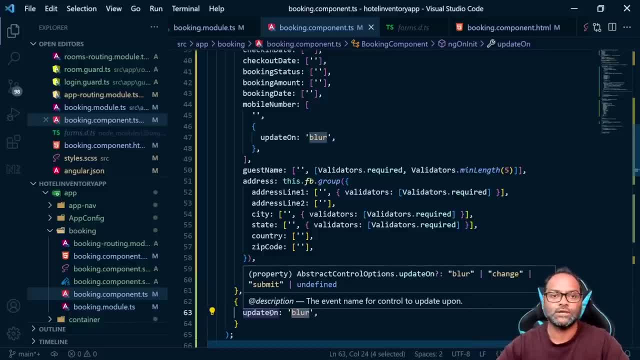 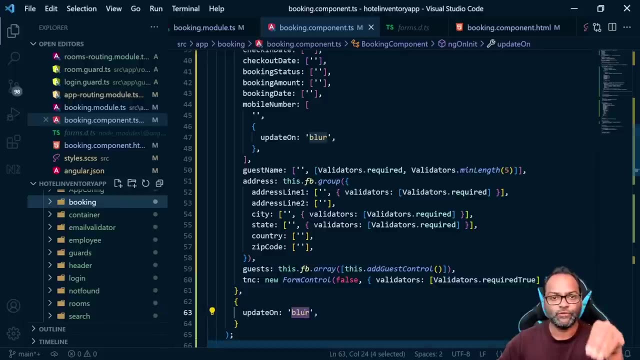 of times or any number of values, only 10 times. your changes will be called on. the control value changes submit one events you might be wondering. I mean, is it possible to control? uh, the same for template driven forms? yes, it is, I just wanted to wait till this time to let you. 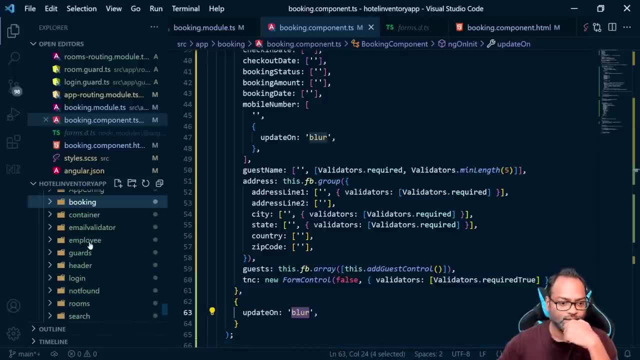 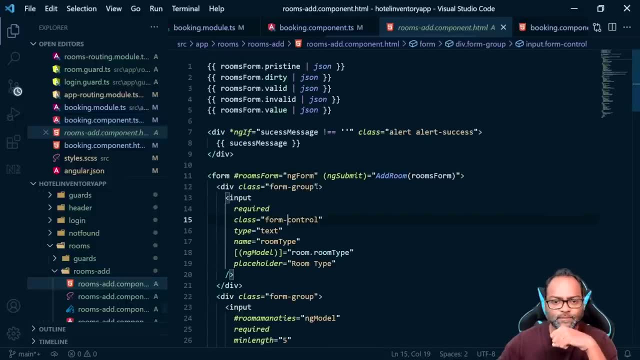 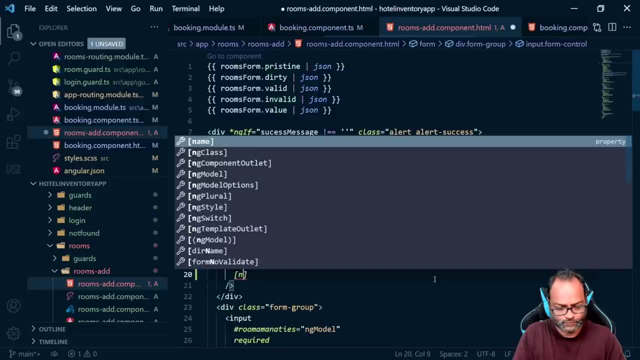 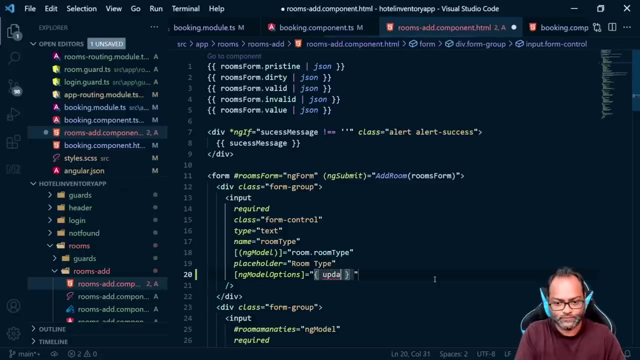 know that, okay, this is possible for template driven forms as well, and to do that we will go to rooms: add here. so, uh, we can use ng model options here where you can pass the properties so you can say update on and you can say, okay, this will be less. so this is how you can control it for your 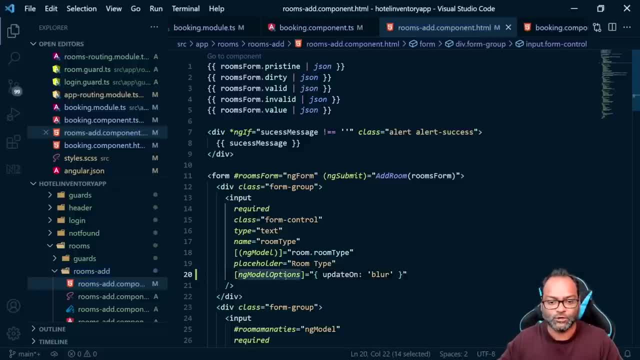 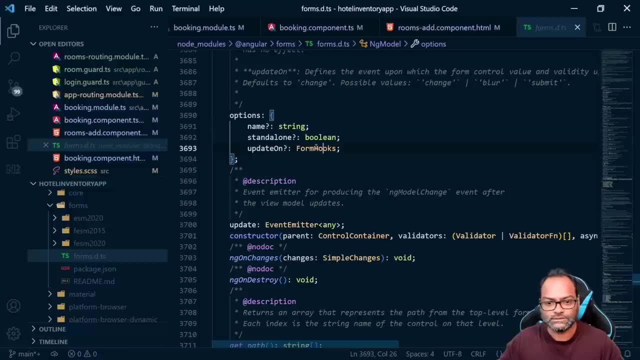 uh template driven forms. so uh remember ng model options and you can see here. so it has three properties. it has name, standalone and update on. so update on uh is referring to these three values, which is change, blur and submit, so you can set it for um or set it to anything you like. yeah, so this. 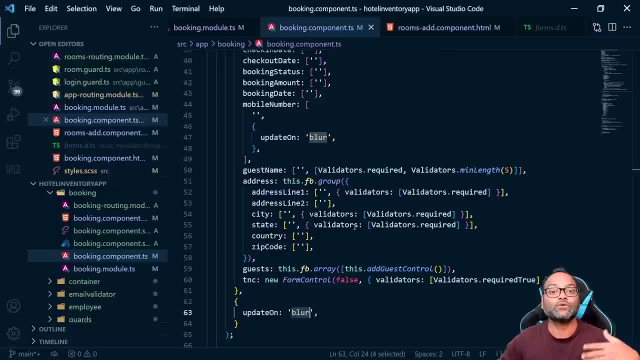 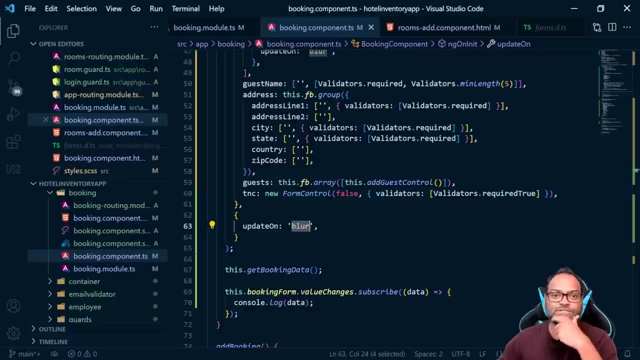 uh. so this is how you can listen to the control value changes and this is how you can also control how you want to listen to those changes. so this, uh, this is it from value changes. now, uh, we can talk about a few rgs operators which we can combine with uh value changes and uh, we'll discuss about. 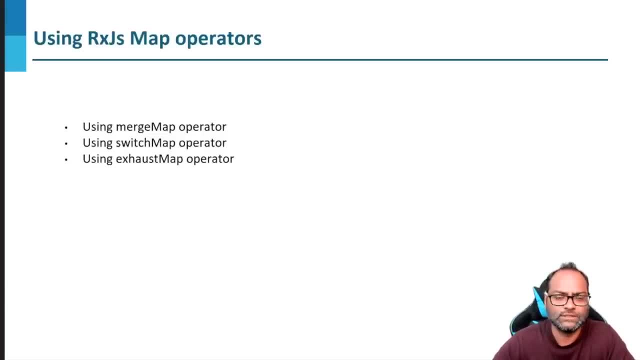 few uh map operators which exist in rxjs, and we'll try to understand each one of them, because it's really useful. uh, in case you are working with rxjs in some big project, so let's go ahead and do that too. the thing is, now we need to connect to a real-time api, and what we will do is we will use. 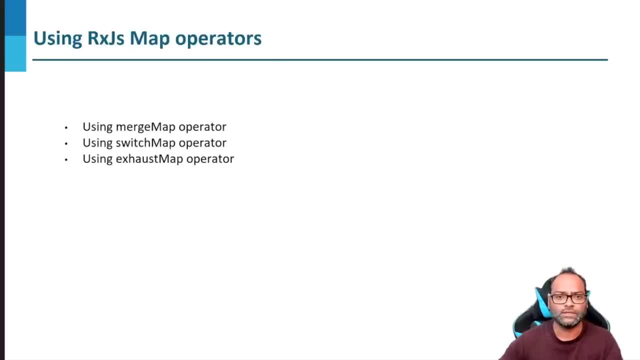 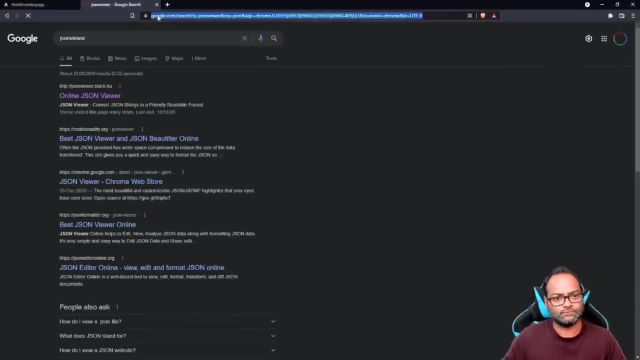 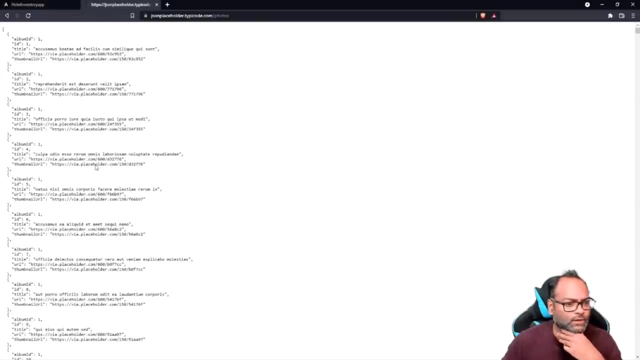 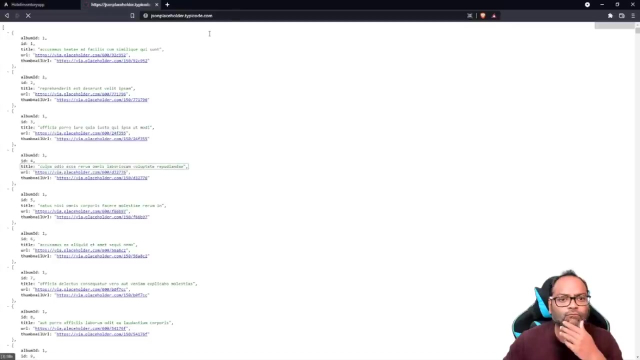 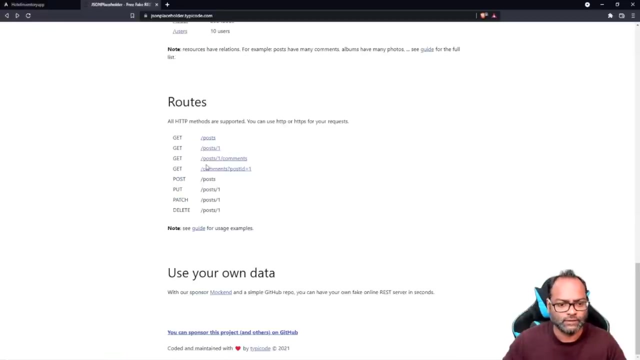 the uh json placeholder api which we used in past because we want to post this data, and in json placeholder actually you can post anything you like foreign. so let's not just in video json placeholder and we'll use post apl and let's see uh, so we can call slash post and that's it. so 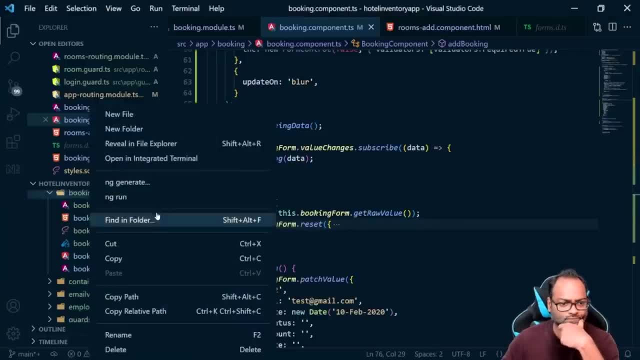 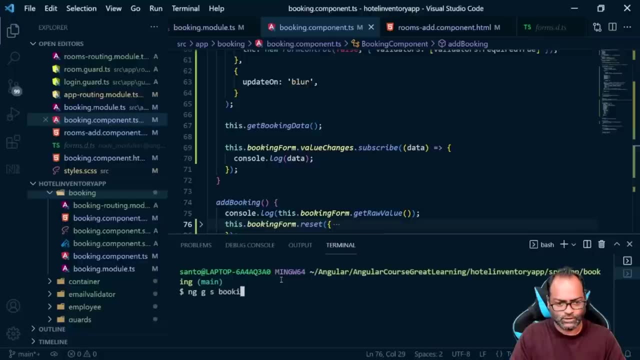 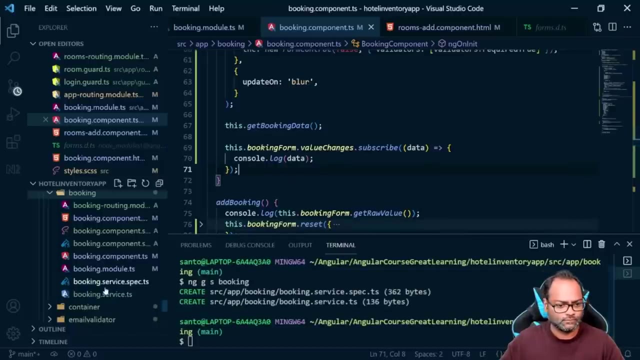 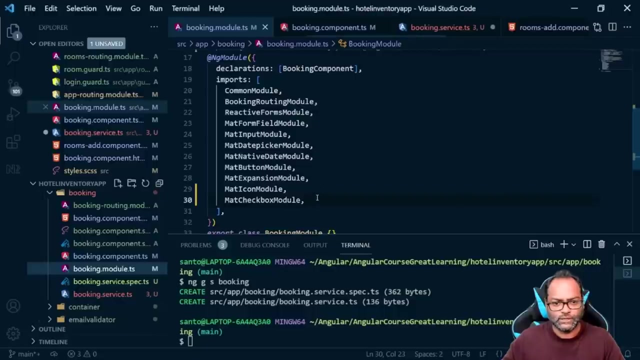 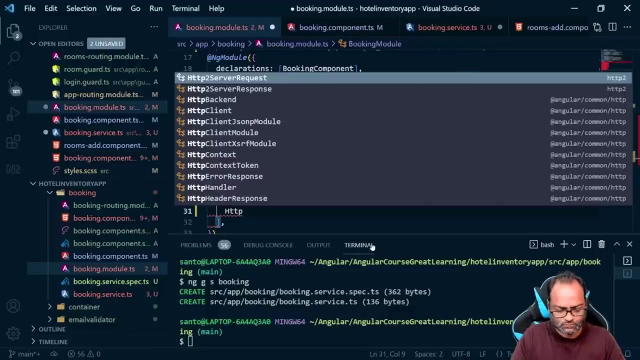 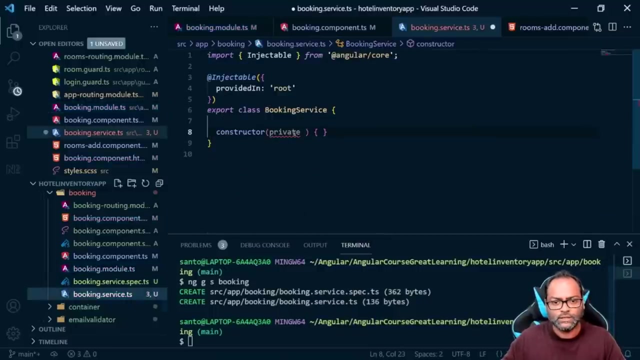 uh, let's go ahead and create a booking service first- i'm going to say ngs and booking service- and we'll use our http service and we also need to register http module. so let's do that http client module and let's save this, and here we will use the s3 service. 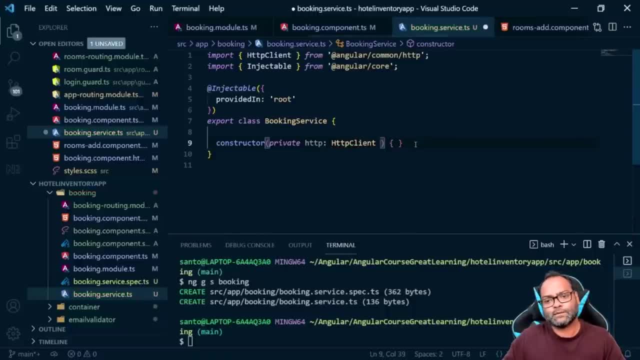 so to be client, and we will say, uh, book room, which is, which has booking data. so right now, i don't, uh, we will not create the interface, so let's do it as any, which we should not. but yeah, i mean, this is anyways, uh, dummy apis, right, so we can say this: 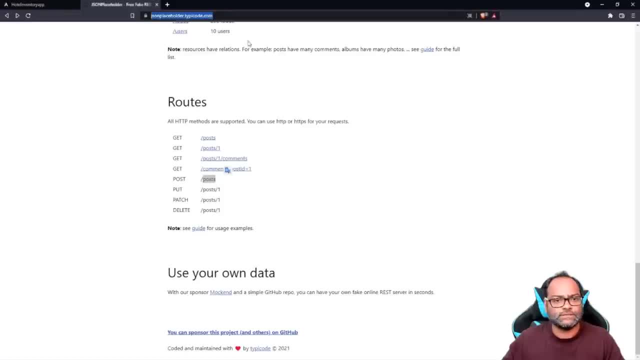 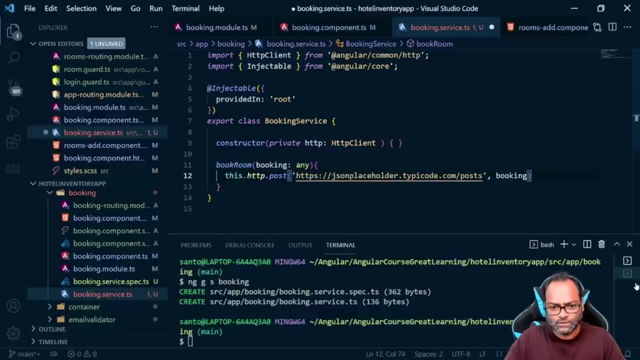 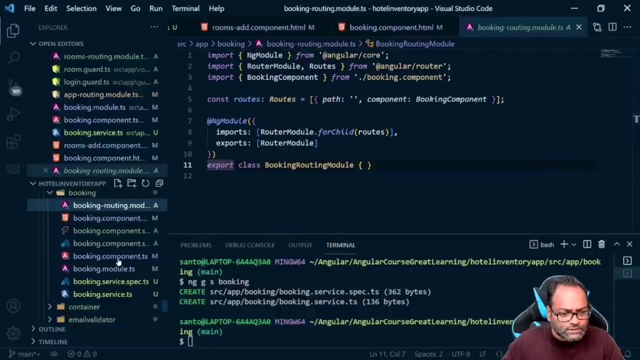 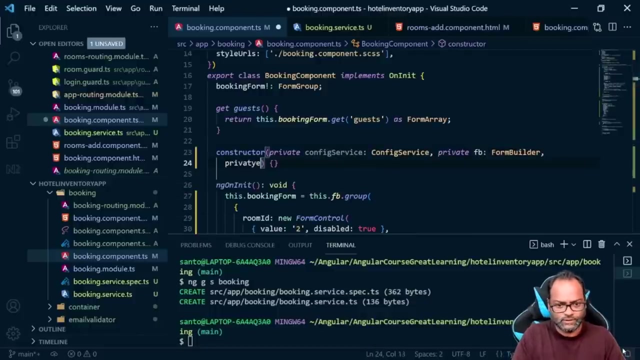 dot, spppost and we will replace this with placeholder json, placeholder uh, slash posts and we'll pass this booking data here and let's remove the subscribe and let's return whatever we get and next we will inject this particular method. where is this component? so it's a private room booking service or just call it as booking. 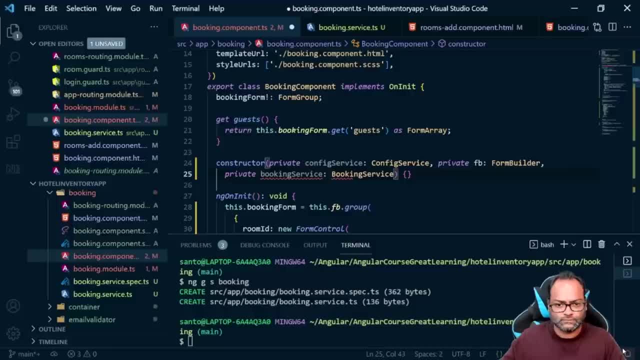 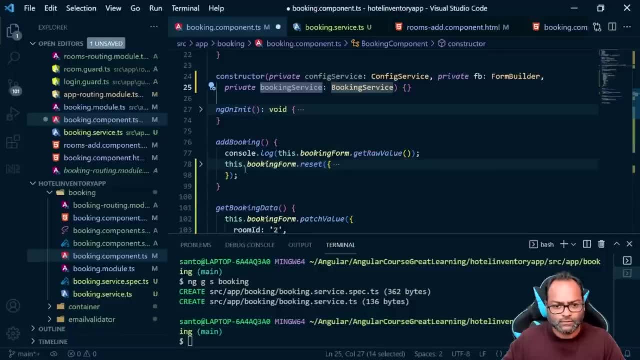 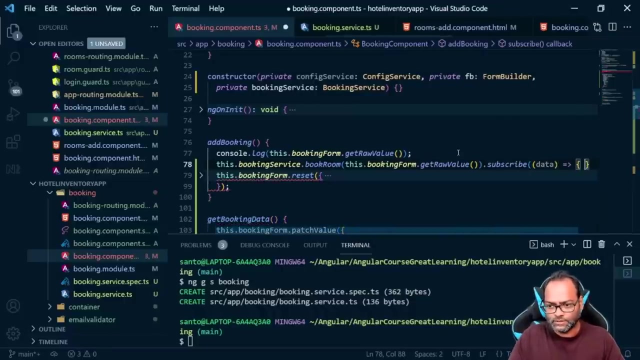 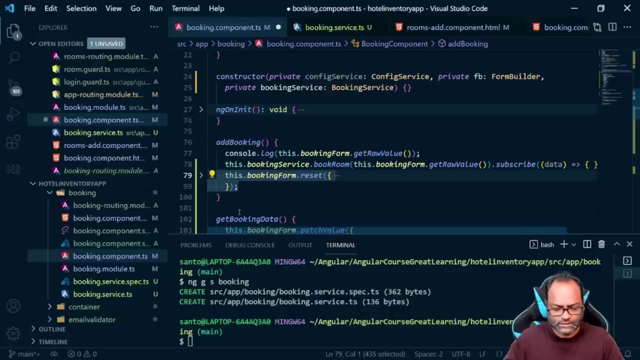 service and we will do it here. so we'll set this dot booking service, dot book room and we'll subscribe to the changes. so let's say this is data and we will listen and we will remove the set reset as of, because we want to see different scenarios. 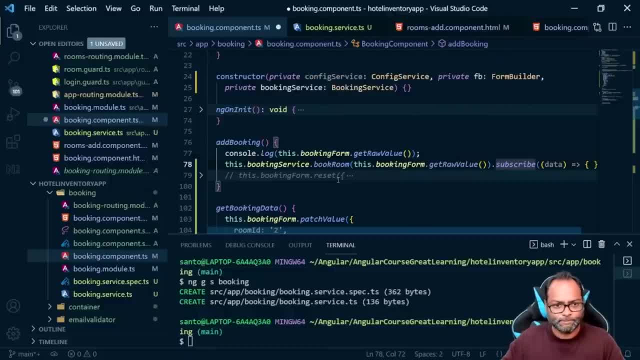 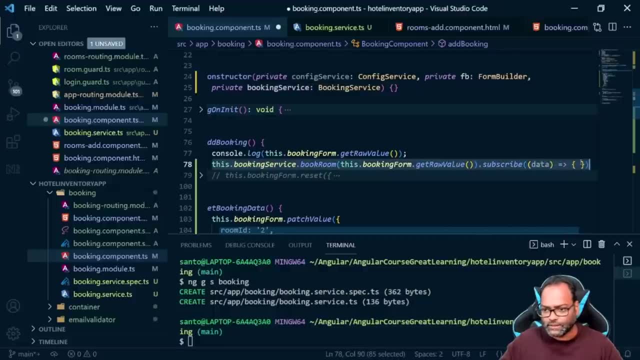 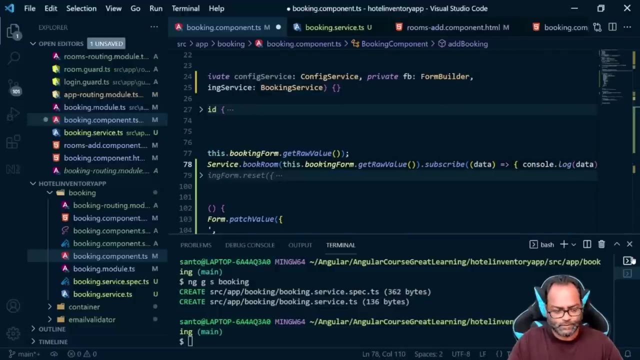 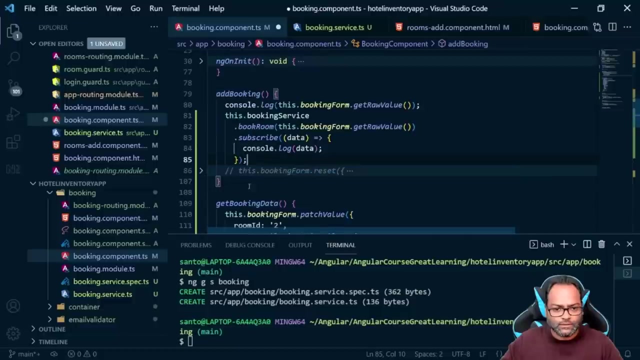 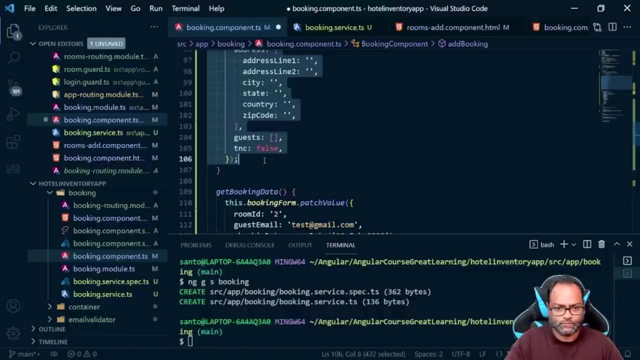 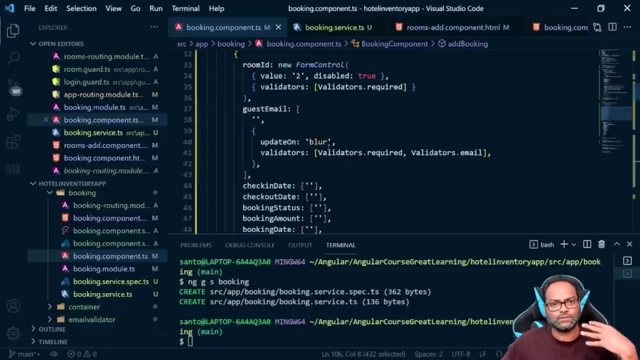 So this is one place and this is on submit, right? So I'll just do console dot log data, which we'll be using in some time, but let's go ahead and control this right now, So to see the example of how this map operator works. 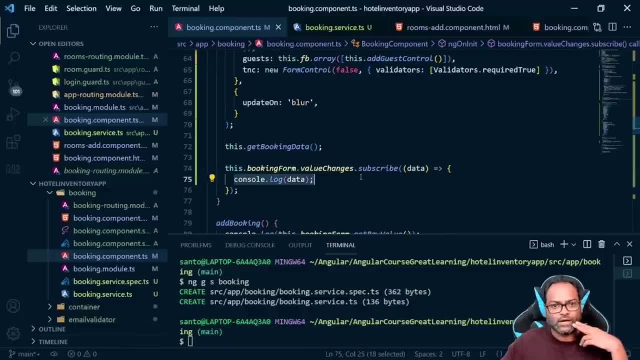 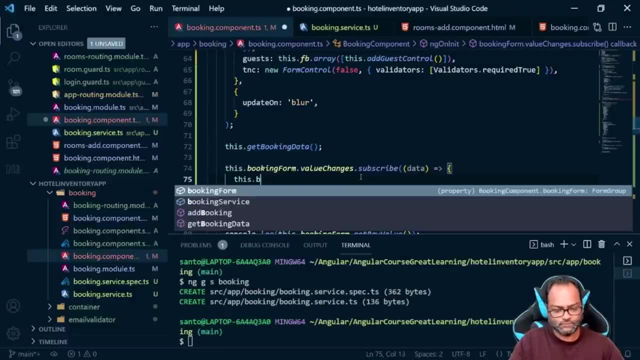 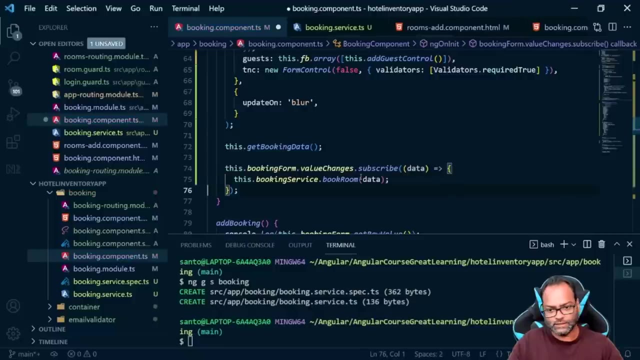 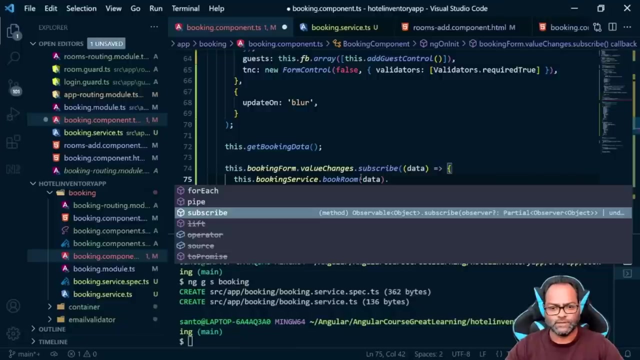 different map operator works. we will be calling our submit method here, Let's see. So I'll say this: dot config booking service, dot book room and we'll pass the data here. So you can see actually what we are doing is we are subscribing, or let's see. 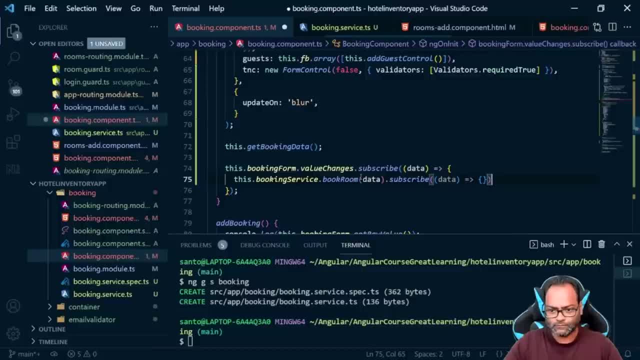 Okay, So what we are doing here is we are subscribing the bookroom method within subscription, which is not a good practice, but we want to actually see the different be different behavior which we have while using the map operator f. So this is not the way we are going to use it. 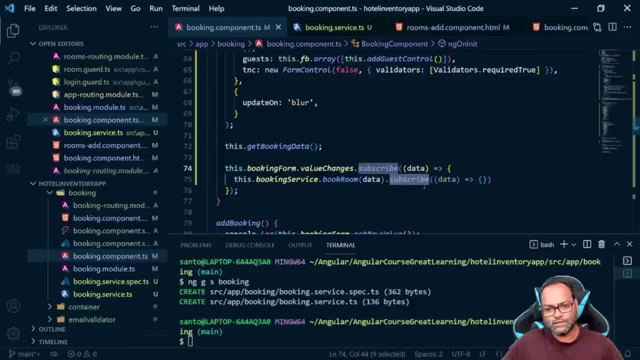 So how we are supposed to do that. So here let's rewrite this and we will be using it, doing it, it via the map operators, so we can do this: dot booking form, dot value changes, dot pipe, and we will be using the different map operators. so let's start with merge map. 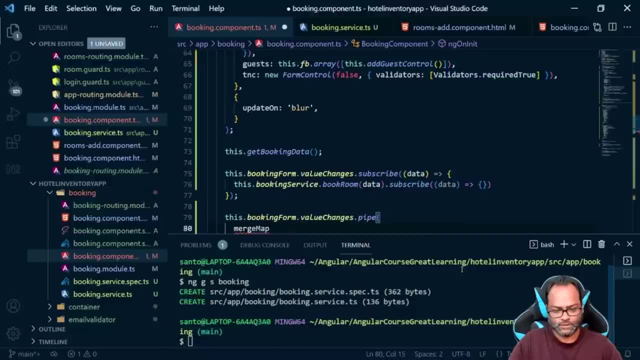 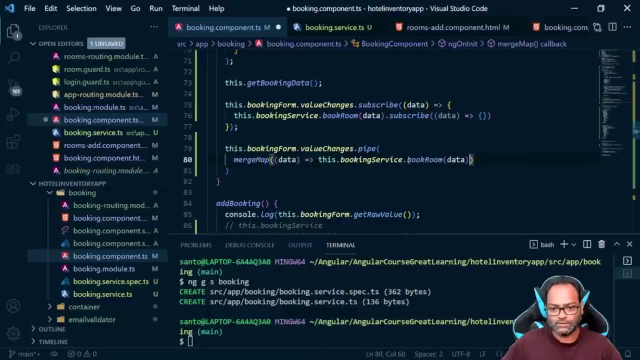 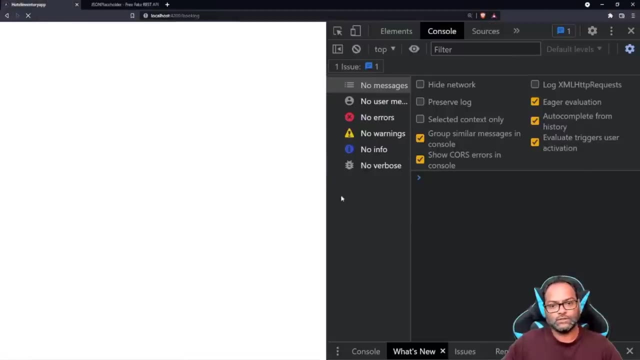 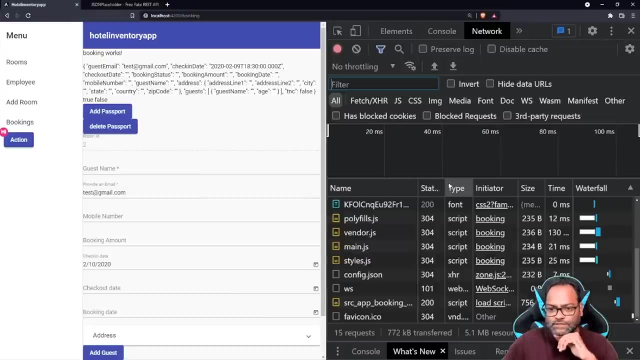 and in merge map we will say, okay, this is data, and then we will be calling this dot book room. let's comment this out and let's see the behavior right now and let's comment: let's remove this and let's go to the network tab, because it will give us. 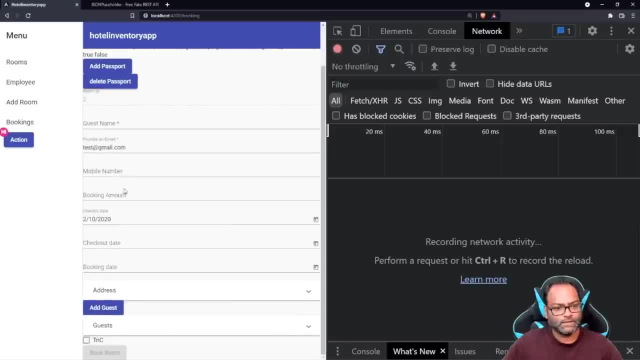 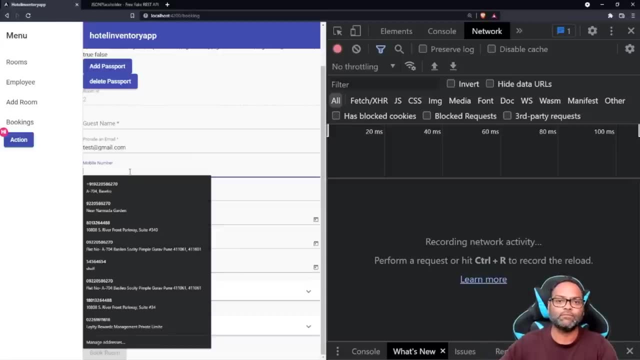 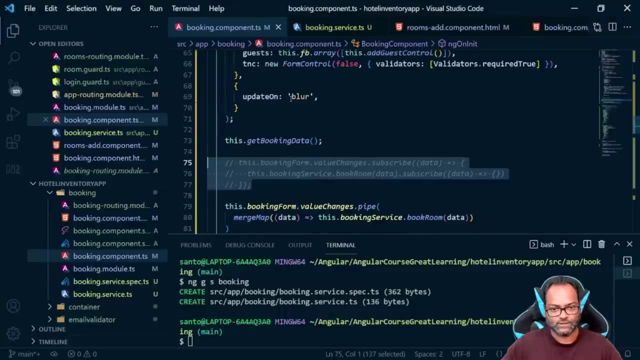 clear idea how the merge map operator works. so remember we have right now. the form will be like: value changes will be called when we move out of the control, because we have sent said the this updated on blur, so let's remove this as well and say, rather than blur, i will go back to. 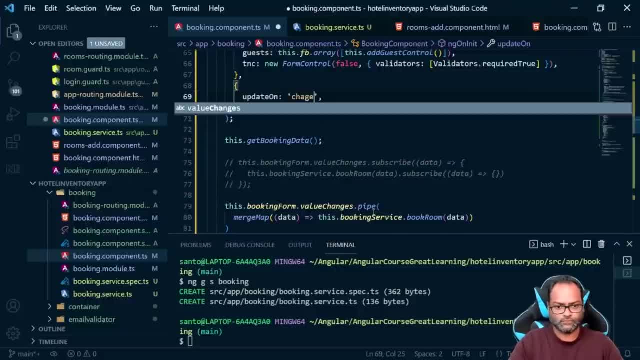 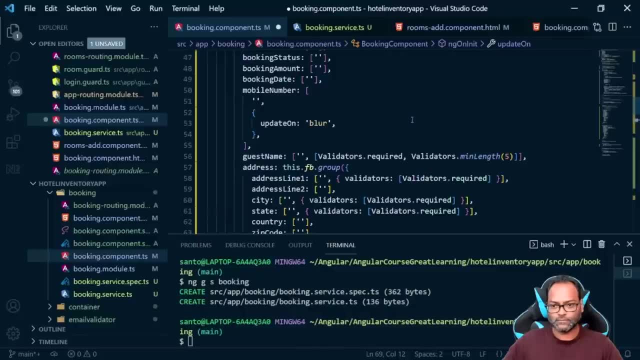 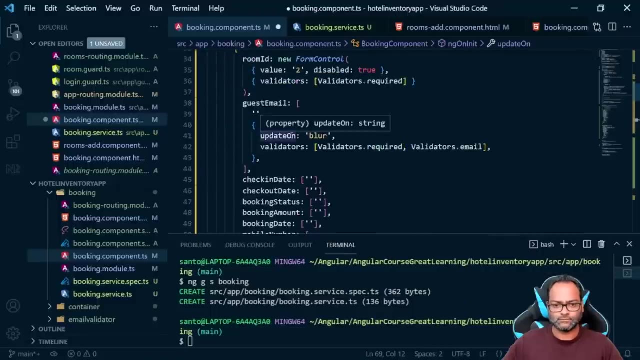 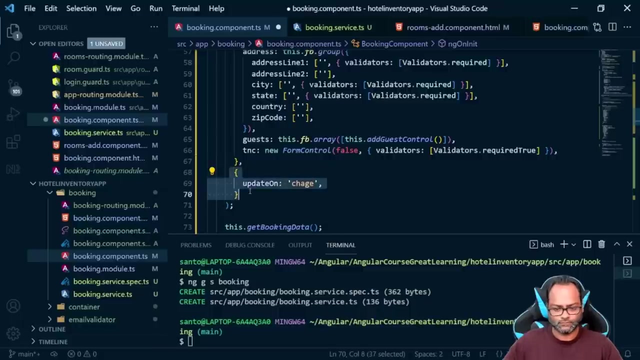 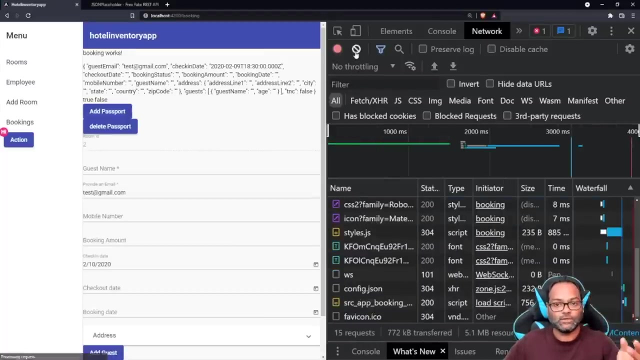 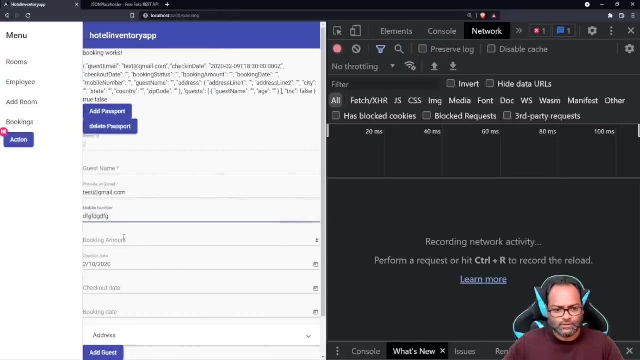 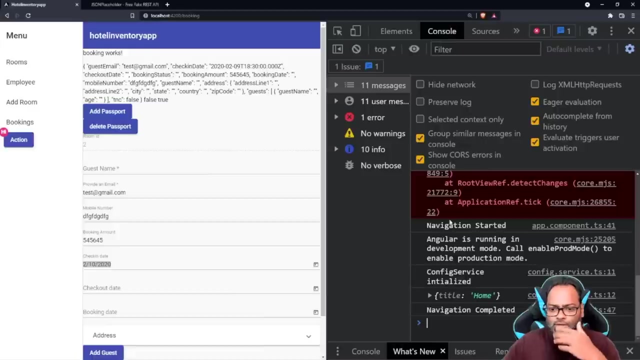 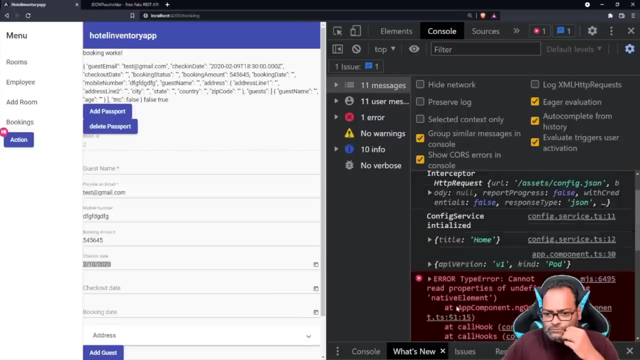 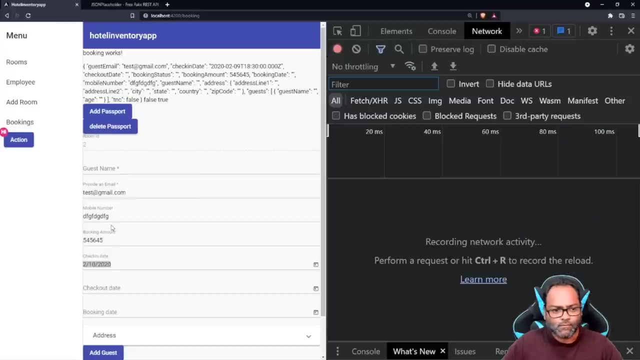 update on: okay, okay, so now, as, uh, we have moved on the default behavior, which is change. let's see how it behaves. so network amount and okay, okay, okay, okay, I'm going to go back to the network tab and let's see what's wrong here. okay, we have not subscribed, so let's do that and let's subscribe to this data. 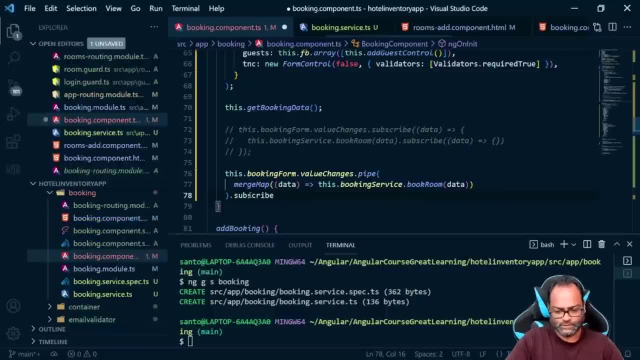 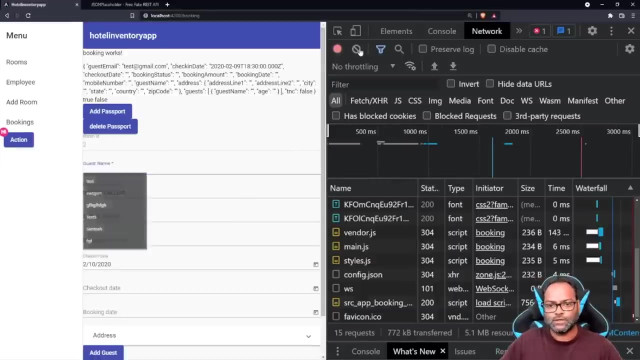 and we'll just do console dot log data. let's see now. so let's go back to this data and we'll just do console dot log data. let's see now, nothing will be called because, as we discussed, I mean, of course we need to subscribe it, otherwise nothing will be called. so let's remove this network. 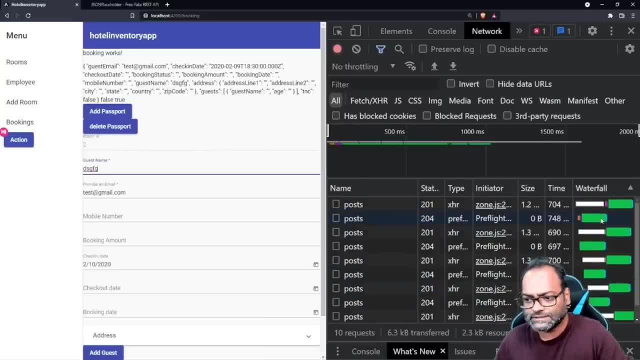 tab and let's enter the guest name and you can see post requests being made in parallel. so you can see it doesn't care. so now trying to understand different merge or merge operators. so first is merge map. so in this case mergemap does not care about the sequence. 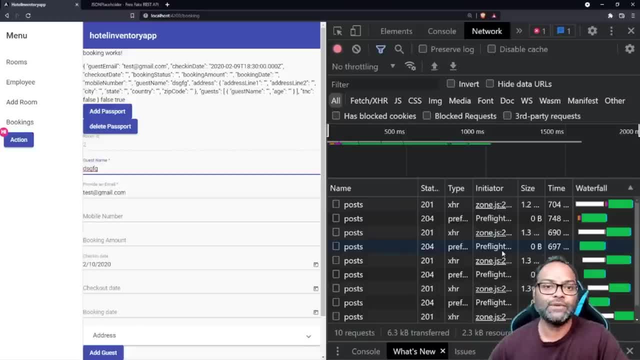 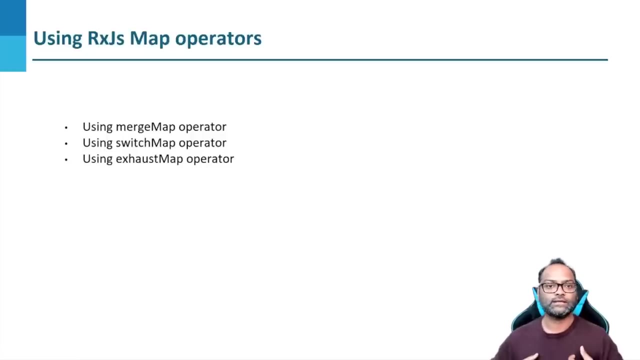 data. or you can say: subscribe to the stream as soon as the data is provided. sequence does not matter, merge map, let's move on to the other operator. so we have merge map which says: okay, i don't care about um the sequence, as soon as i get the data or a stream is. 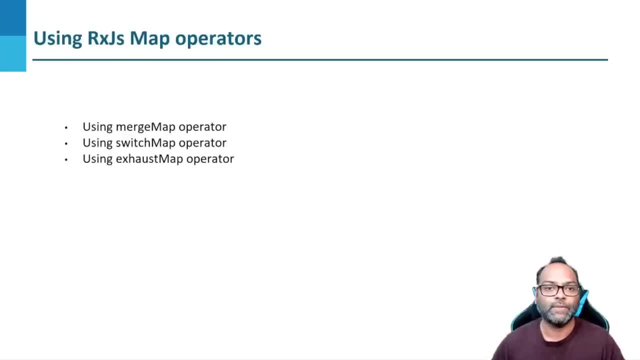 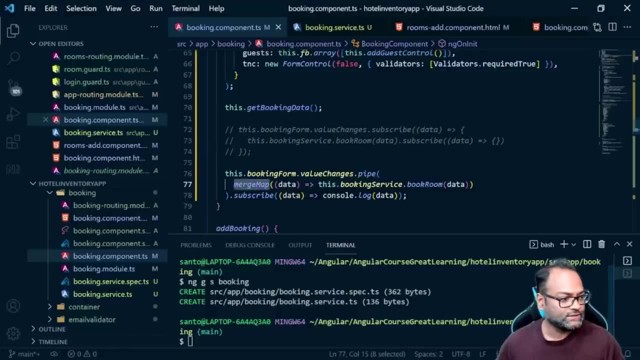 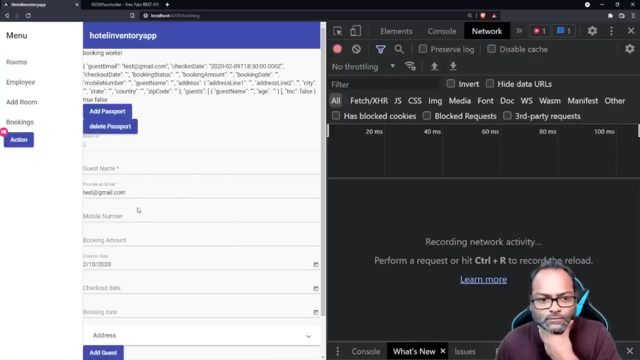 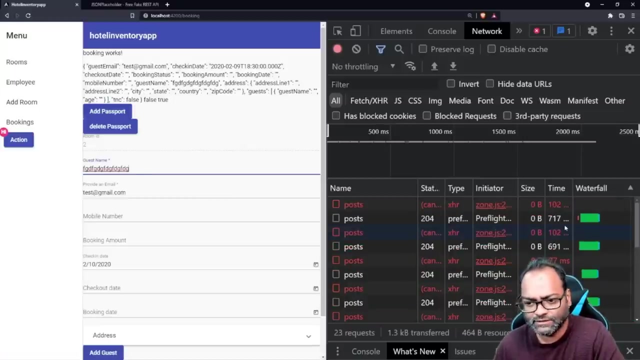 as a stream is emitted, i will just go ahead and pass the stream to whoever has subscribed now. now, next, which we will use: switchmap. let's see how switchman behaves here. network tab: yes, can you see something uh which is different? so let me just explain this behavior now so you can see there are a lot of uh requests. which are being delivered on your mobile independence. now, this is a commercial solution 嗹. the one that i want you to see first are which is making teclations and um, the popular which are being produced at site github. one at github now, this is modernized teqlat. you can see those. are in search in wordpress keyword per page for using that. if you add that information, you'll need to. so i'm just emergingcek to make a non zoom search. that is what we will use it to save your time. so you will be looking at black magic watchers. 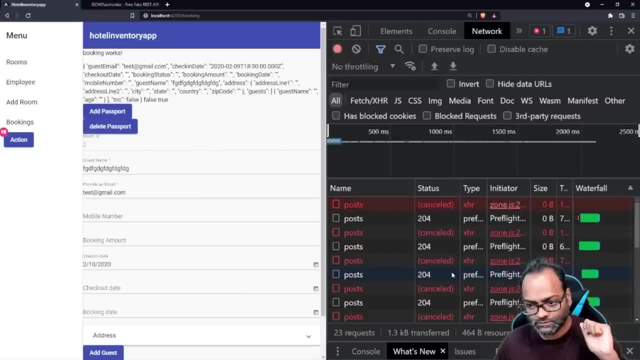 canceled. but what is happening here? so in case of this switch map, switch map will wait. sorry, switch map will cancel any existing request if it receives a new data. so let's say, if you care about that, whoever has subscribed to your stream should get the latest data only and should previous. 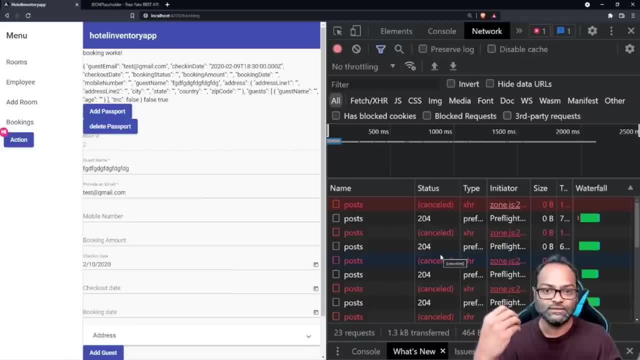 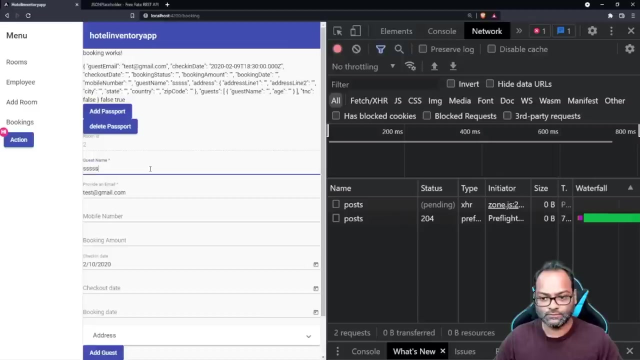 data or previous stream which is raised should be cancelled. you switch map operator is the way to go. now let's talk about the last one, which is exhaust map. let's enter. you can see I entered multiple characters. exhaust map cares about the sequence, so it says until unless the previous request is not completed. 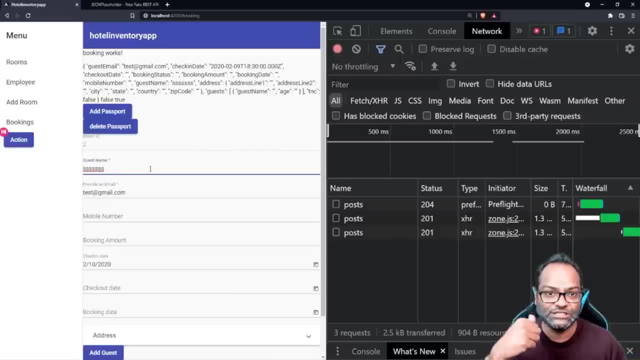 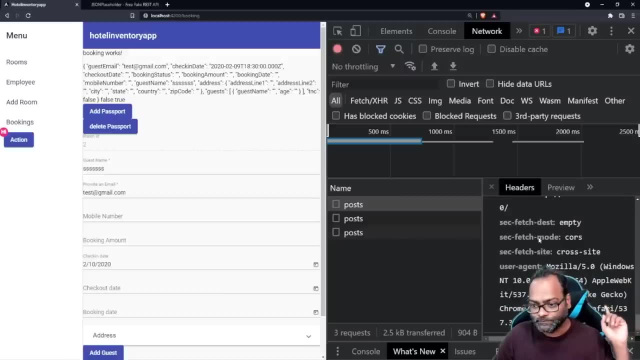 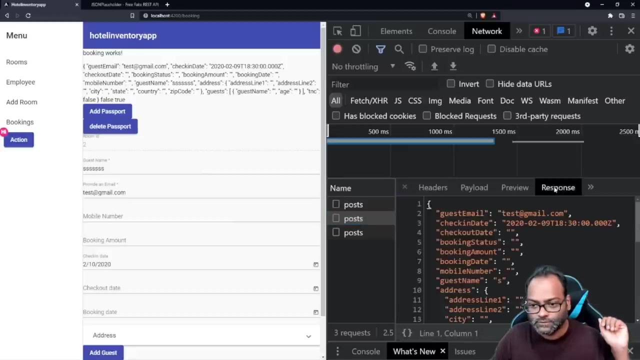 I will not subscribe to any latest changes so it takes its time to complete the previous one. so you can see it has. so here you will see the data. now let's talk about request header, response and right. so you have your data available here. so it says okay, until unless the previous request. 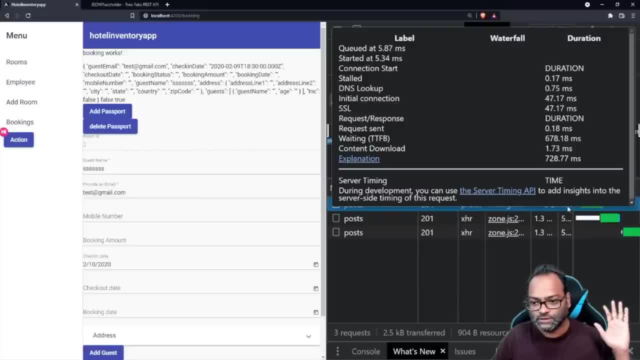 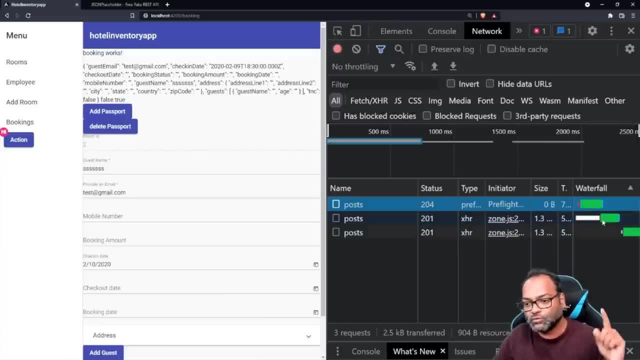 is not completed. I'm not going to call anything else. so this this API is. I think it was never called, but you can see here. so this API started here. it says 204. okay, so these are two APIs which are called. you can see the first API request and you will be able to see the values request header. 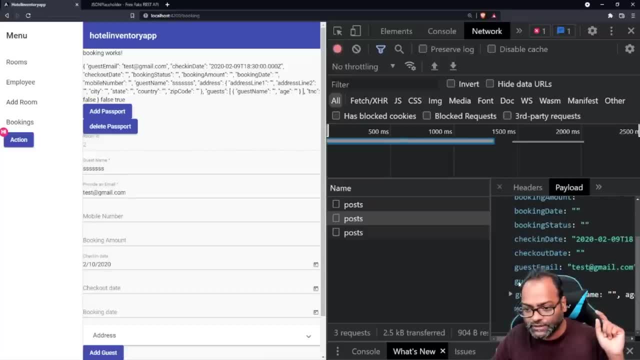 response: header payload where you have all the data. so we entered the guest name and then it waited until unless this request was completed to make the second request so you can see the rest of the values actually went into second request. so in case you care that, okay, the previous request which you made should be completed before I can. 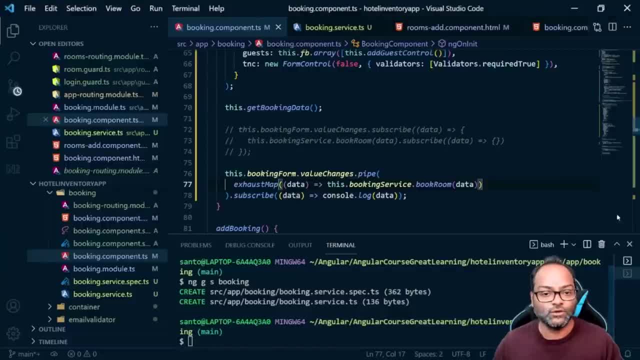 make a new request. this exhaust map is your operator which you are looking at. so we discussed about three map operators which are really useful. as I said, you don't have to use all the operators, like more than 100 operators which exist. you have to remember list 10 operators. 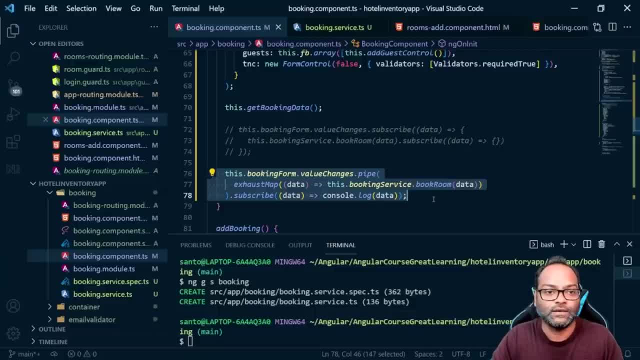 which we have already used in this particular, in this particular course. and if you use all these operators, if you master all these operators, it's more than enough and once you move or once you get more scenarios, you can actually explore more operators. but you don't have to start like learning. 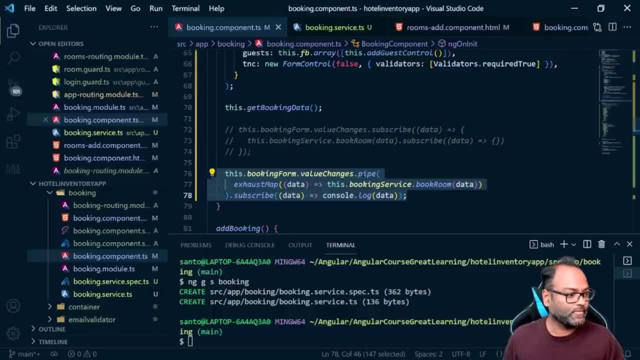 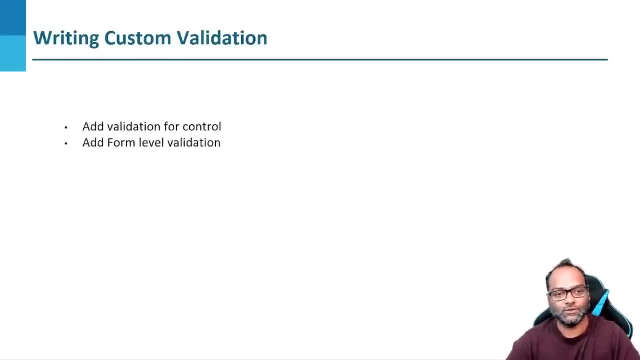 100 operators on day one. now we will talk about how to write custom validation for reactive forms. so we will learn how we can add validation for control and we'll also see how we can add validation for form level- which is a little bit interesting because you may get this issue- and I'll talk about few scenarios where actually this is useful. 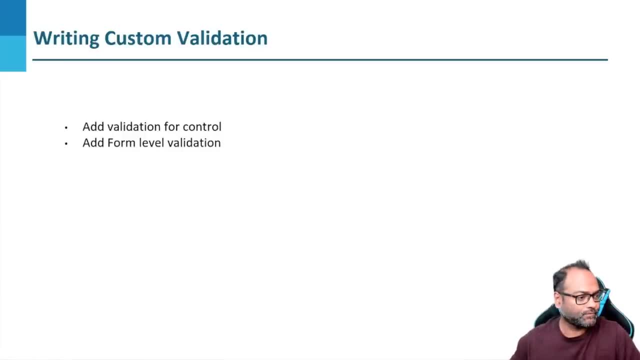 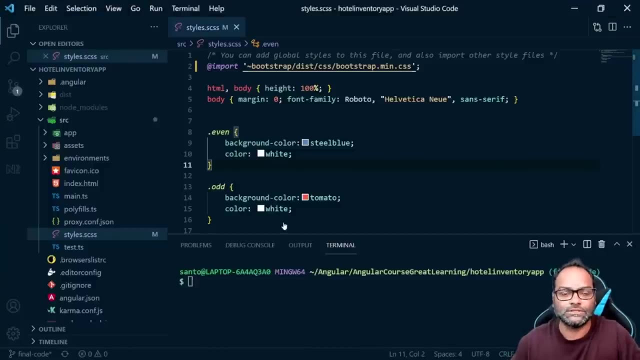 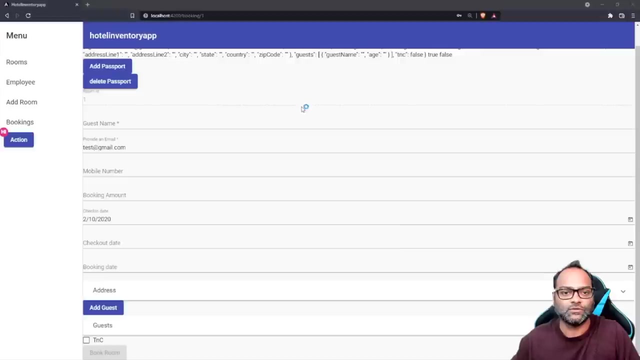 but before we do that, let me just start. before we do that. remember last time we got some issue and we had to disable bootstrap. so what I have done is we have just added this, we have actually enabled this input, which seems to fix the issue, where both angular material and bootstrap seems to work. so 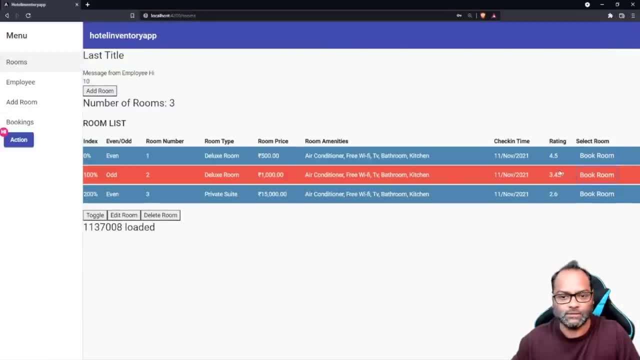 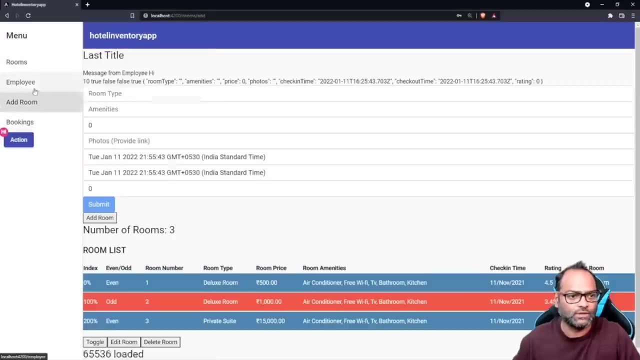 if you see, this is the form and this is the table, right, so it both works. we'll also do one more thing. we will do little bit cleanup because we, if you see- I mean on all the pages- we have a lot of junk data, for example this which we use just to just to uh. 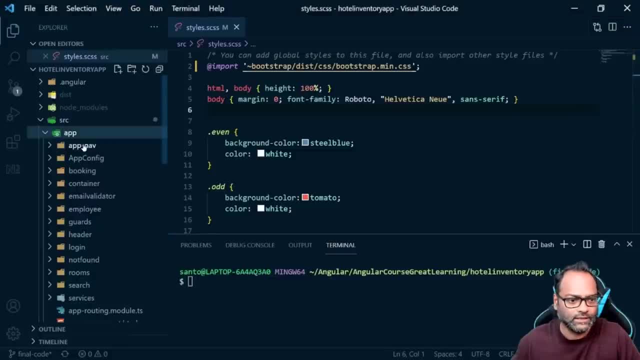 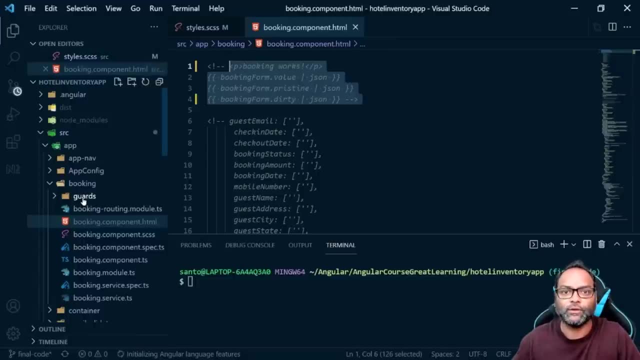 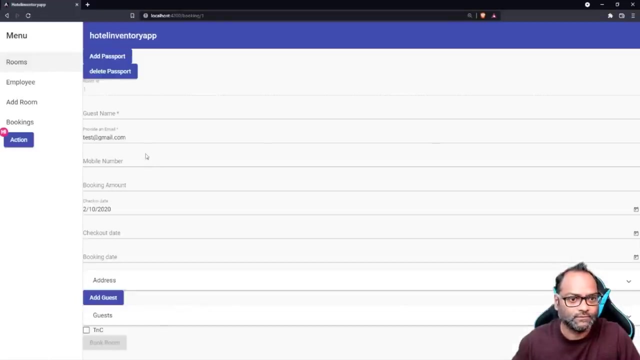 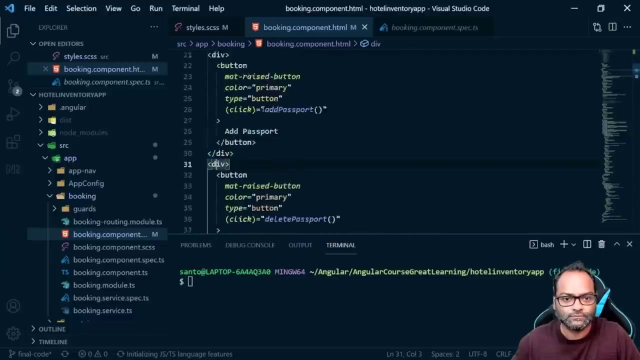 show you right how the data looks like. so let's go ahead and clear those first, and then we'll move ahead. so I'll just- I'll just keep it here- it's not like I'm going to remove it- so you can always refer: uh, these values and gone, and let's do one more thing. 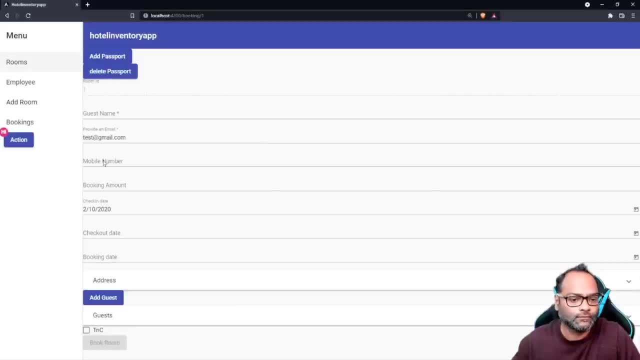 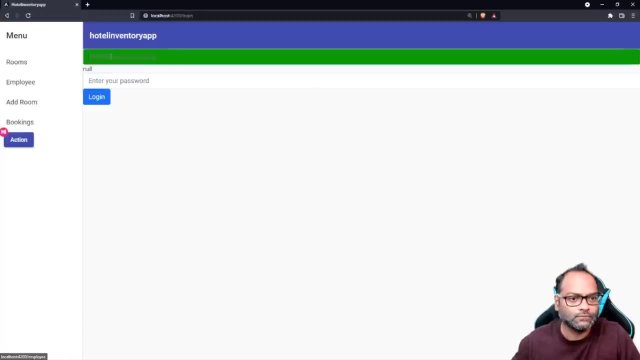 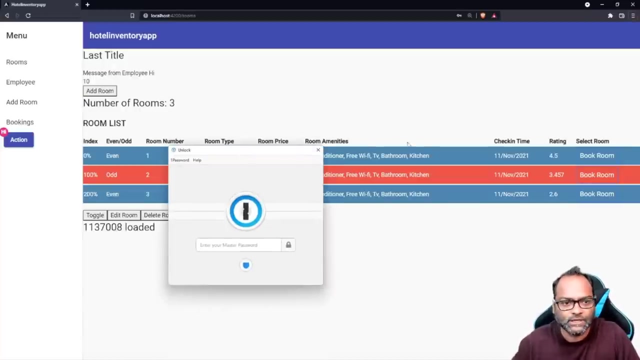 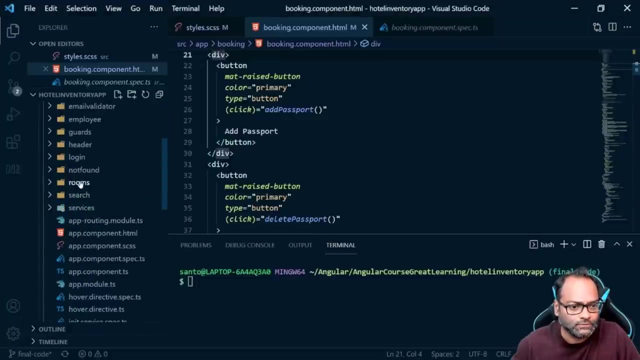 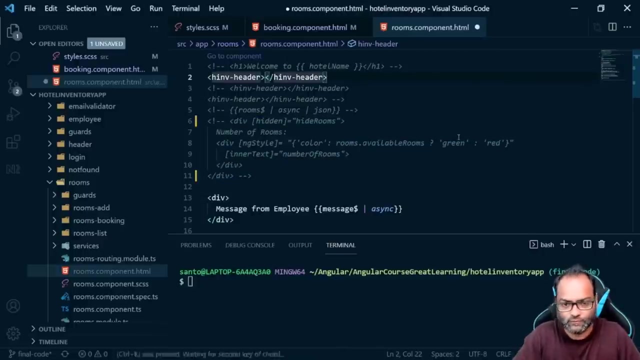 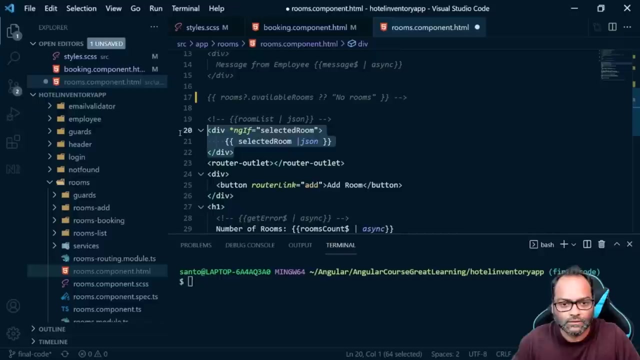 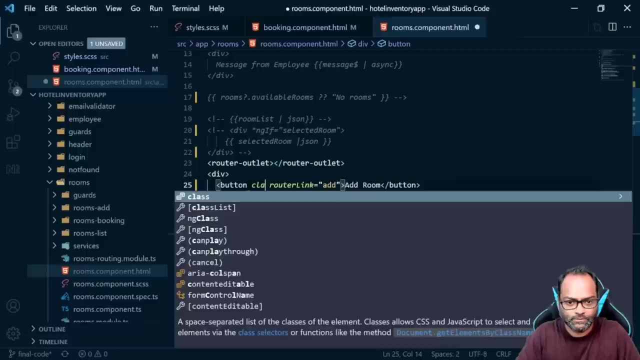 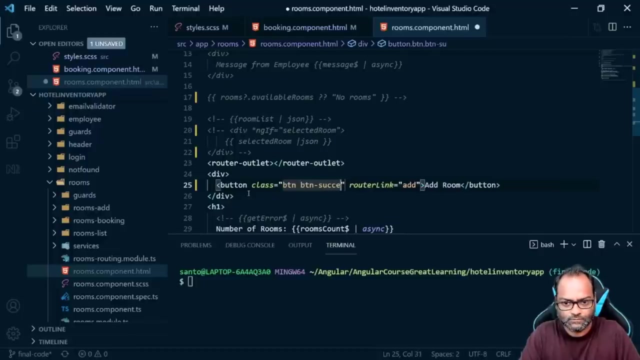 so let's clear this as well. uh, we'll just keep the table. that's it. so this is our rooms component. so let's get rid of this. let's remove this. let's remove this and let's keep. keep this and we will use between between success: let's remove. 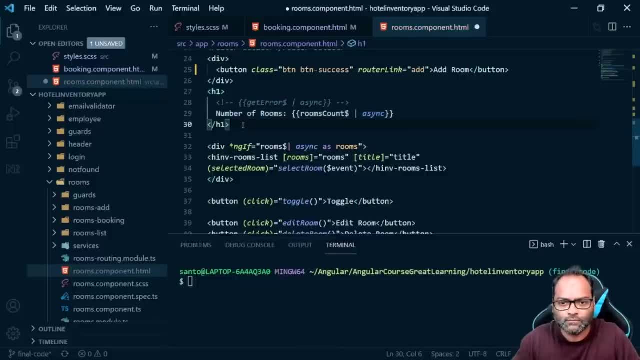 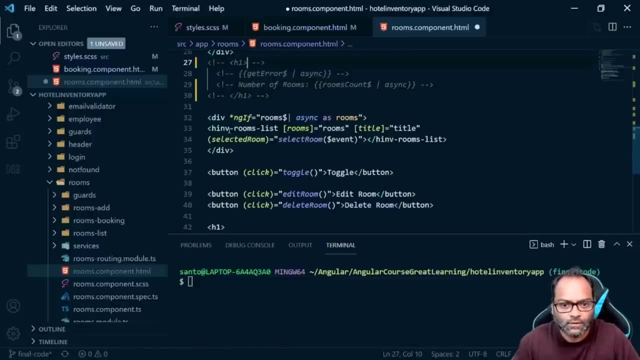 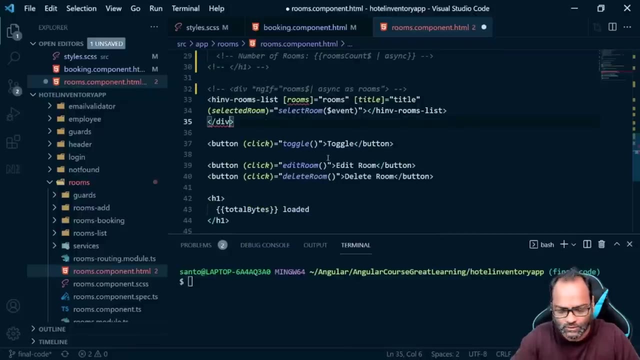 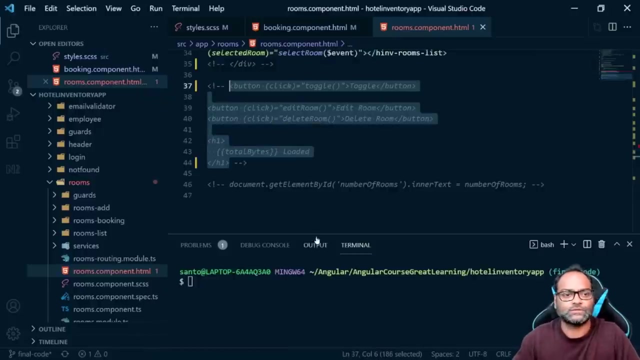 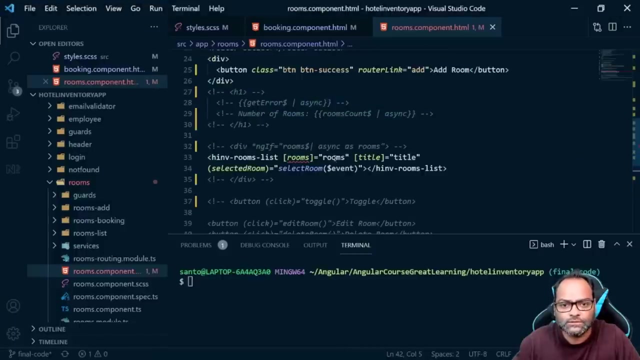 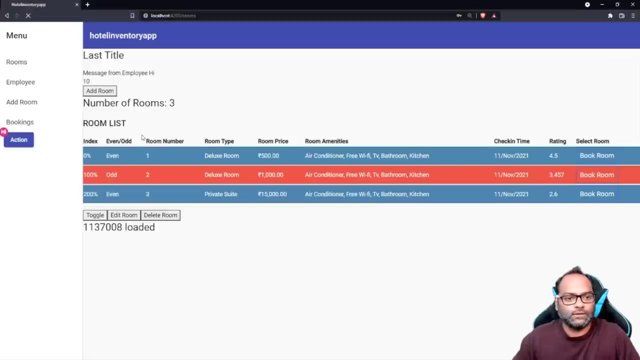 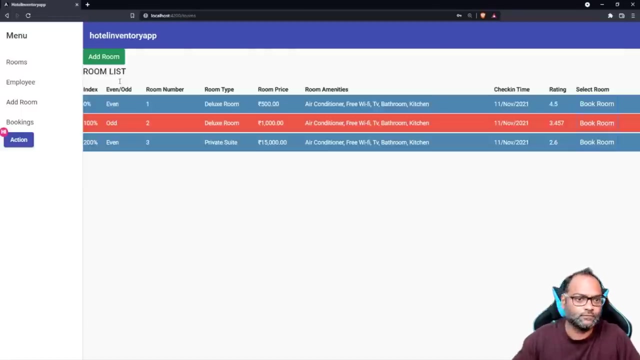 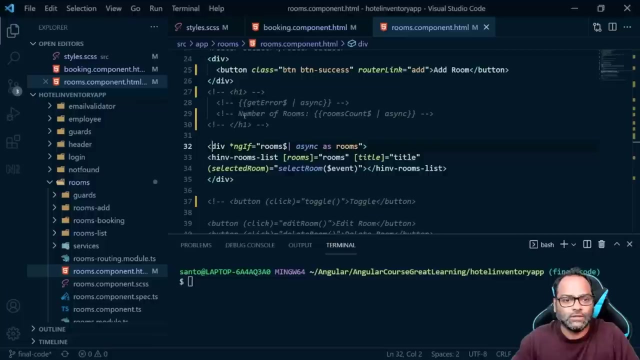 sorry, we'll keep rooms list there- there isn't being okay- and we'll disable these buttons too. let's see room is missing following property rooms list. uh, okay, and looks a little bit better, right? I mean, now we don't have a lot of junk uh data which is available here right now, and let's comment this one too. 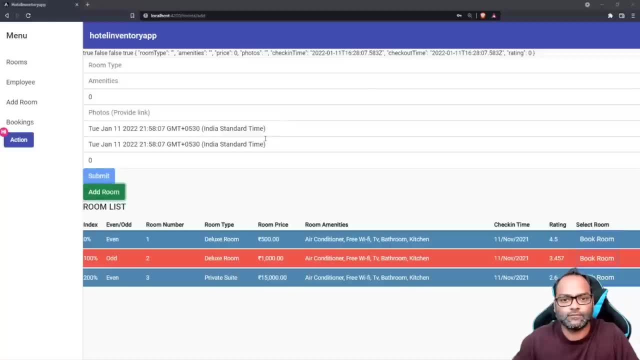 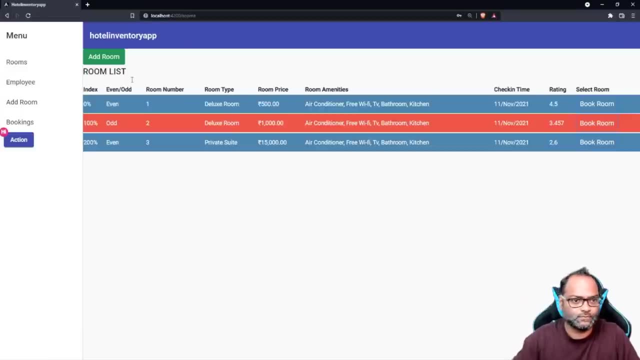 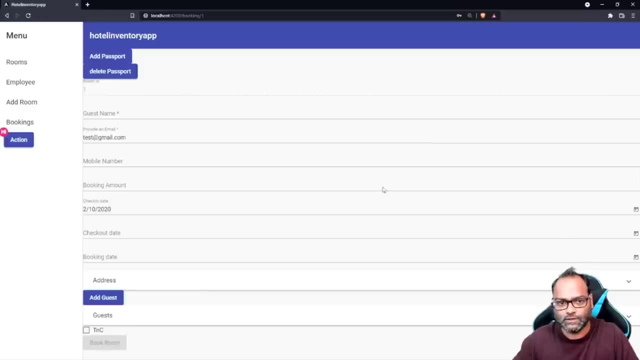 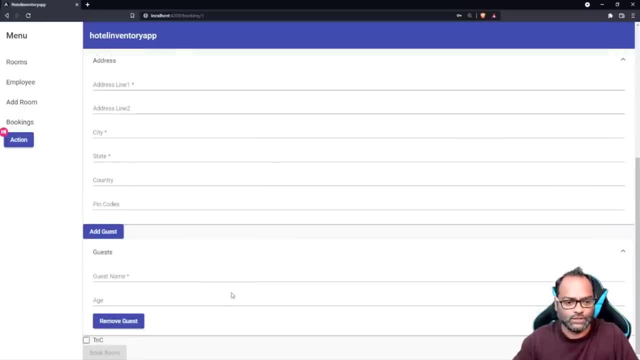 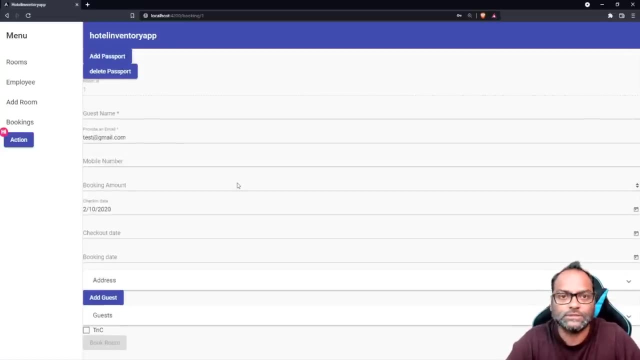 book room, and this is the book room component which is available here. so what we will do is: let's go ahead and add few custom decorators- sorry, not because sorry. uh, let's go ahead and add some custom validations to this reactive form and let's see what are the different ways in which. 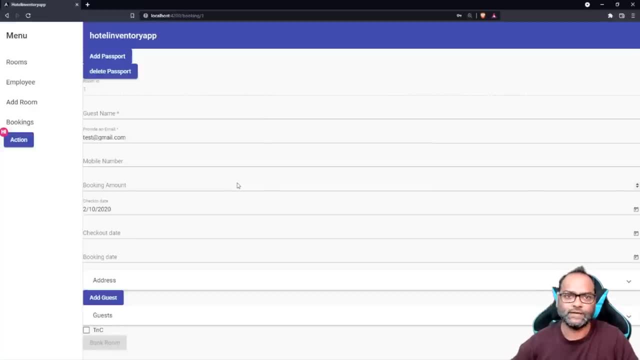 we can do that. so let's start with a simple validator, where what we will do is: we will validate a control, let's say, example, guest name. same, same scenario which we'll take. remember in uh, we we wrote a custom validator where we said: okay, in case there is a test in. 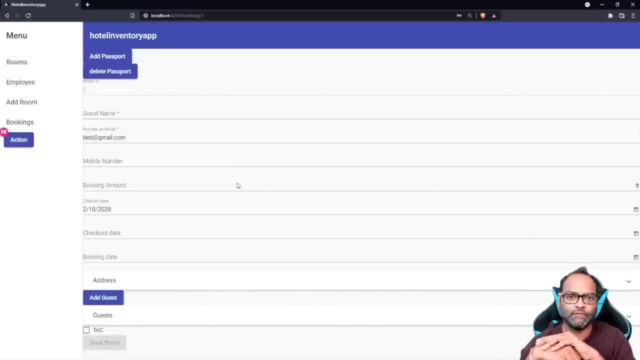 name: uh, go ahead and reject this particular value. so it should show the validation that, okay, the name is invalid. same, we'll do it for guest. so we'll add a validation, but using the custom: uh sorry, reactive. uh, well, i mean. so we'll add a validation where we'll say: okay, in case this. 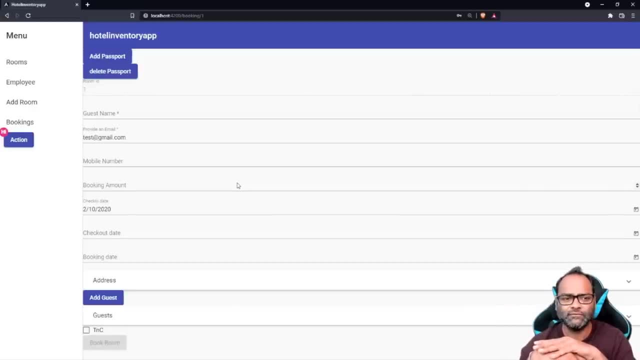 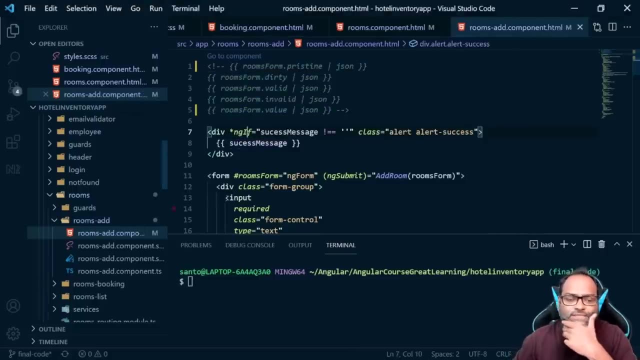 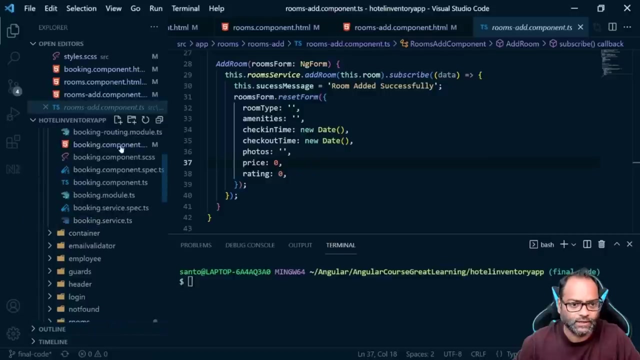 name contains value as test, we will just uh give a validation error. how to do that? so i generally try to follow the same approach, which is uh followed by validators class. so let's go back to the booking and booking component and remember we have already used some validation rights. 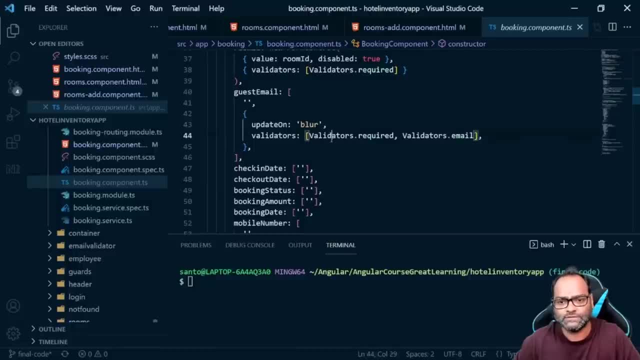 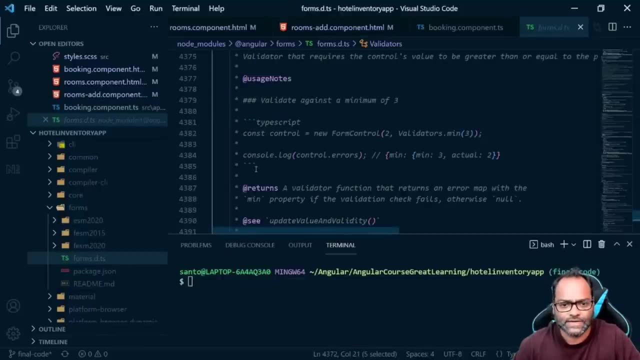 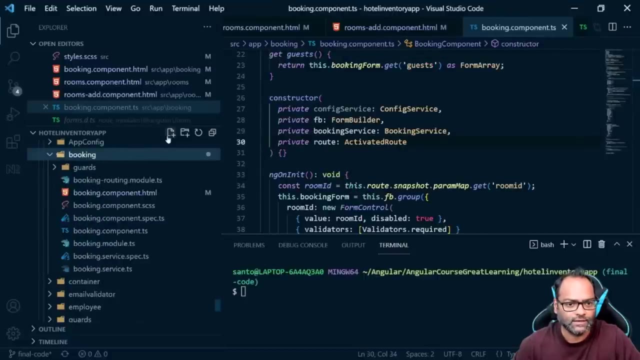 so we have added the built-in validation right now, which is which uses this: validatorsrequire- validatorsemail. if you see the implementation of validators class, it's a class with some static methods, so we'll try to follow the same approach and to do to do that, let's go ahead and add a. 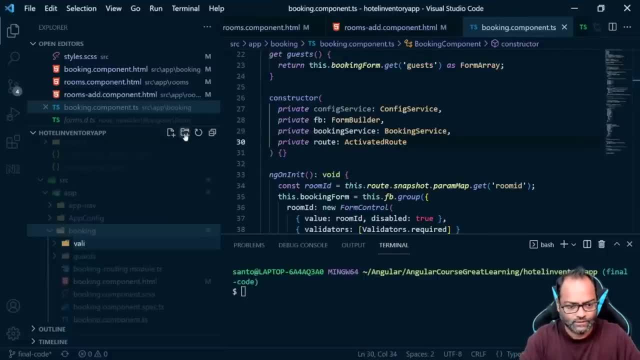 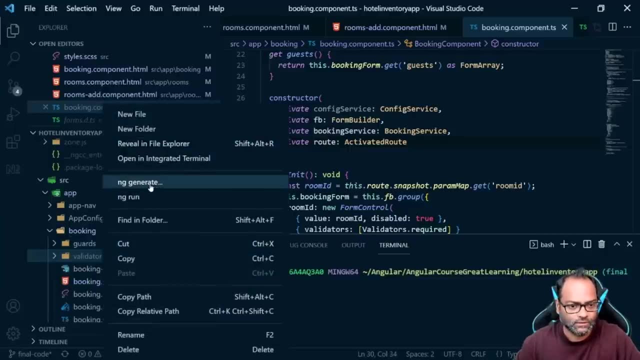 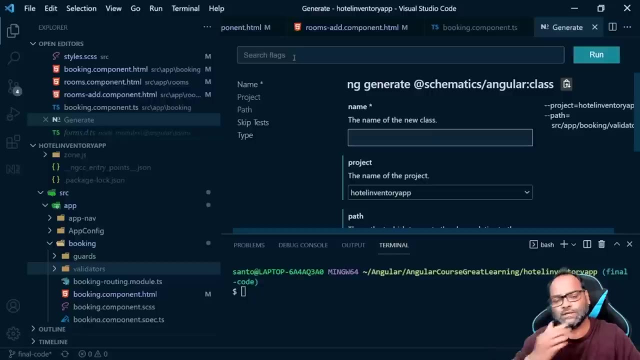 folder, we'll call it as valley directors and let's create a class. so let's see ng generate. if it has a class i'm using. uh, this is okay, let me just show. uh, talk about this as well, and i have added an extension for called nx console, which lets you do that. so, um, i'll just say this class name is: 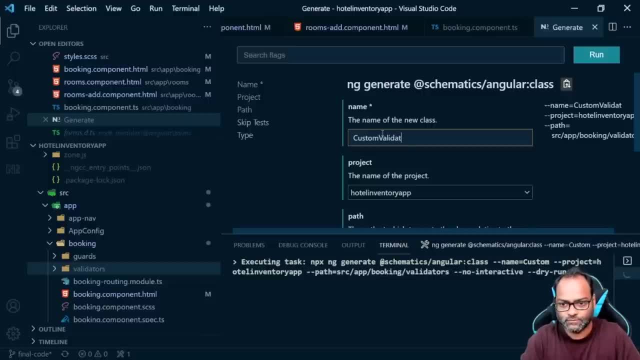 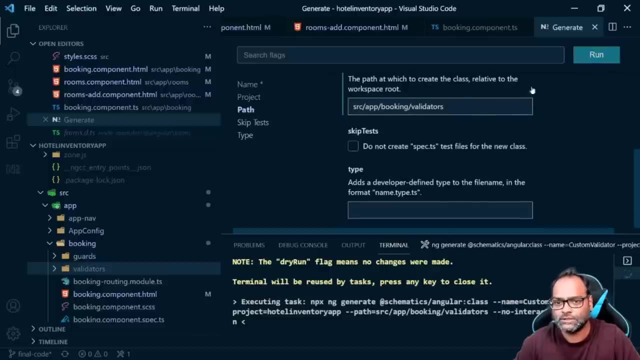 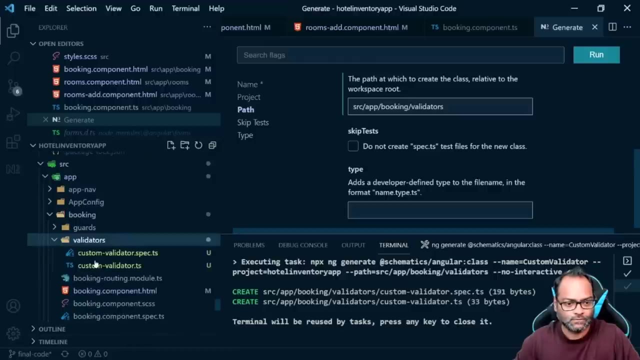 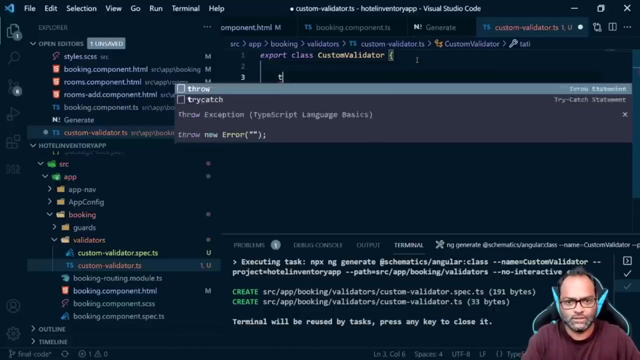 custom valley data and project name is fine. this is the folder where i want to do it and that's it. and we have this class created and here we will add some static methods. so let's add some very data. we will be adding all the very papers in this particular file. so i'll say this is a validate. 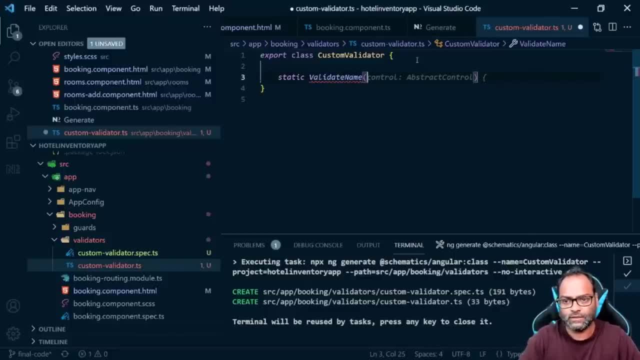 value, date, name, and so let's talk about this now. so we have a validate, validate name function and it takes a parameter called abstract control. so what is this? abstract control is? so? abstract control is base class for everything: form, group, form control, form array. so it's a base class, so it knows it has. 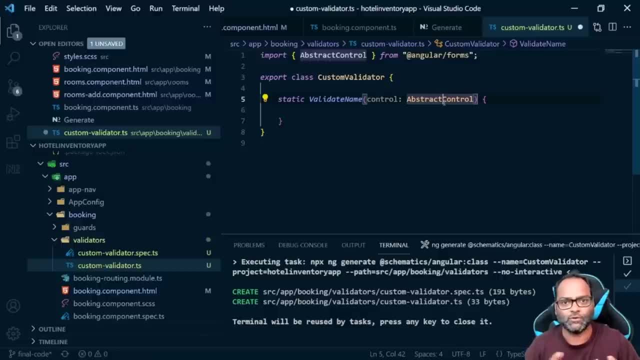 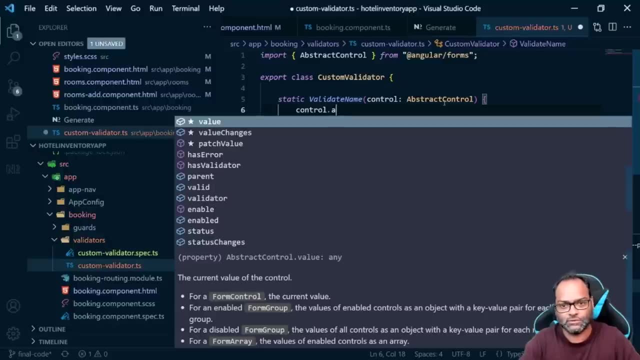 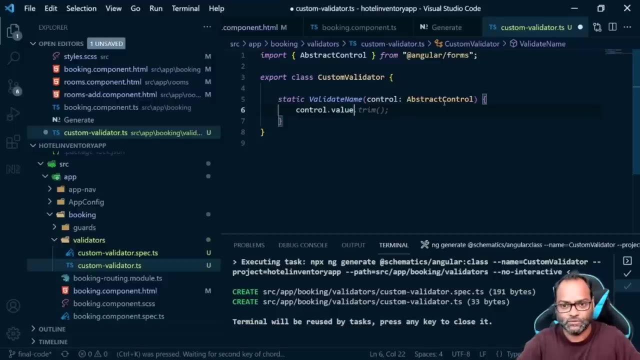 all the information which your all form control form group can have and you can get the value by using: so control dot, value, so this, this will give you uh, the value, uh, which, which, which is entered into the control right. so let's try to validate name. so, first thing, first thing. 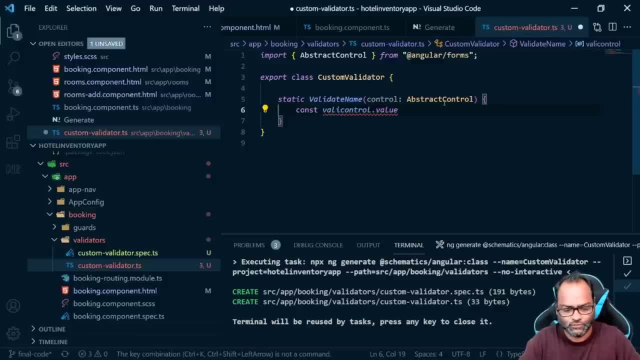 which we'll do is i'll say const value is equals to control dot value as a string because, uh, if you see, the value is actually type of any and i need some uh, as we know that, we know that, okay, this uh name is going to be string, so we are type casting it as a string and we'll say: if 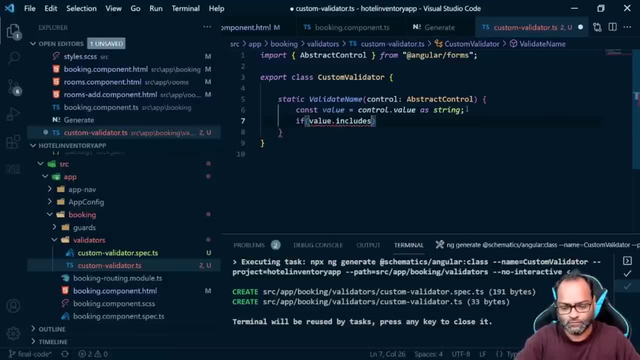 value dot includes test and it's the same. so if remember uh, we can return an object in case there is an error. so i can. i can say validate uh, not this one. i can say it returned in valid name, true, and if this is not the scenario, return null. so once you return null, it means there. 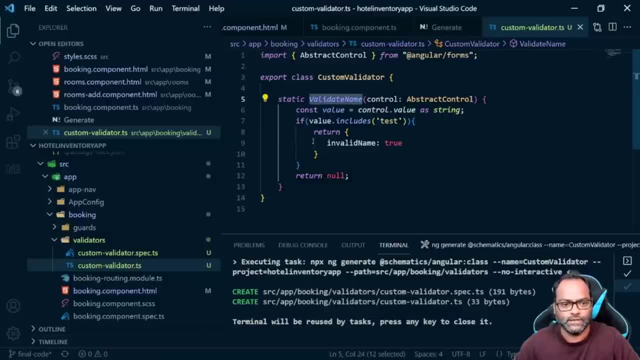 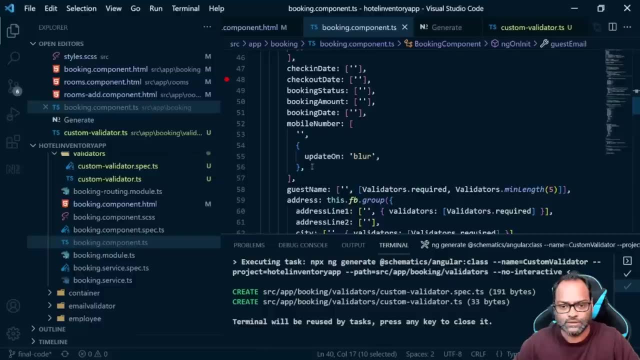 are any Moore's laws. and if you return null, it means the value of the value of the value S and no validation error. and let's see how to apply this validator now. so we can go to our component and we want to apply this to name. so let's see where the name is. this is where, and you can add: 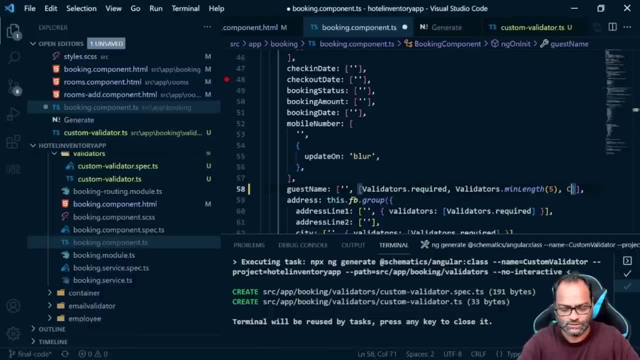 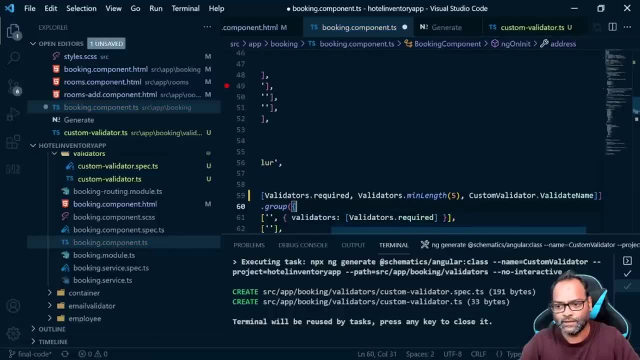 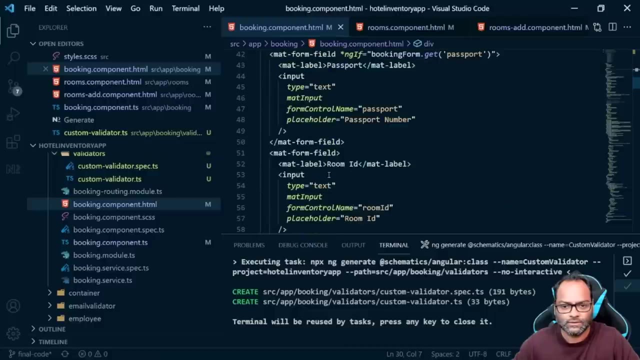 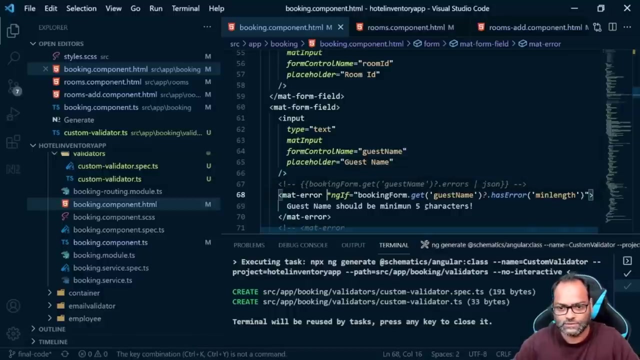 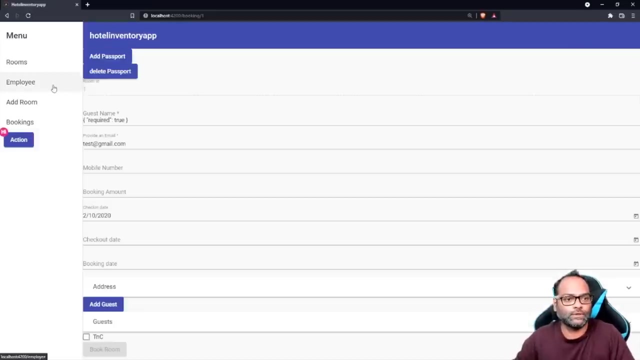 your validator in this list of array, so you can say, okay, this is custom validator, dot, validate name, and let's go ahead and see save this. and here let's go to the name: guess name. right, so we will enable this to see, uh, the list of errors which we have, and let's go ahead and say login. 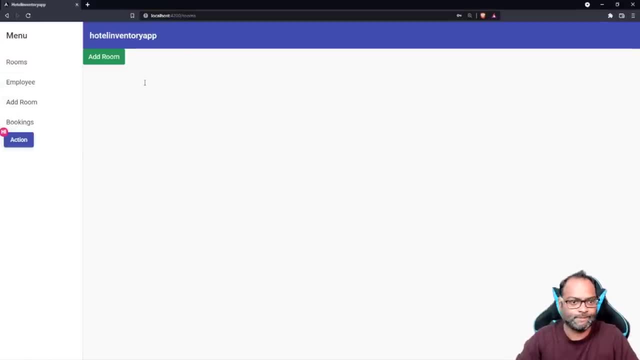 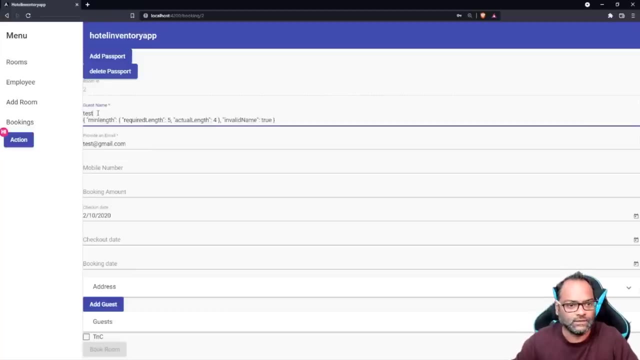 sorry, select the room, and here we are, and let's enter a name which has like test, so you can see invalid name, true, so, uh, now this is. this is the simple validator which we also wrote for uh, template driven forms, so where we are just checking if this particular text exists. 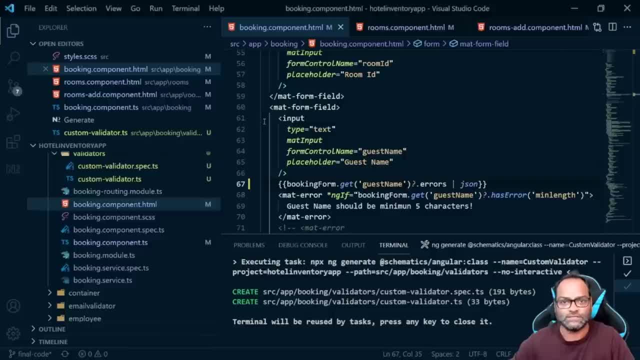 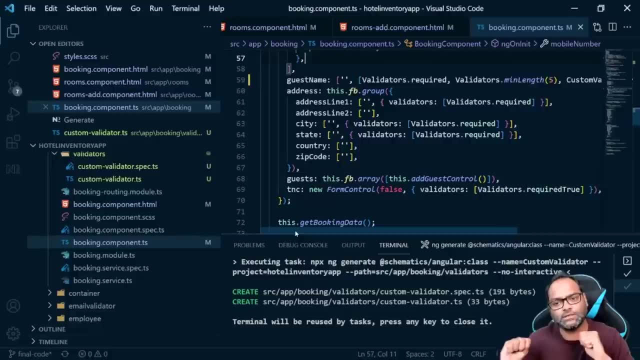 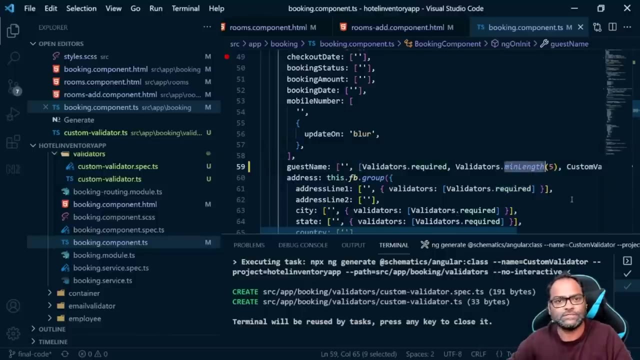 in this particular control. just go ahead and give this in validation message. so now the next validator which we will write is something where we can pass some value. so it's like let's see here: right, so you have min length and we wanted to pass how much the length should be, so we'll 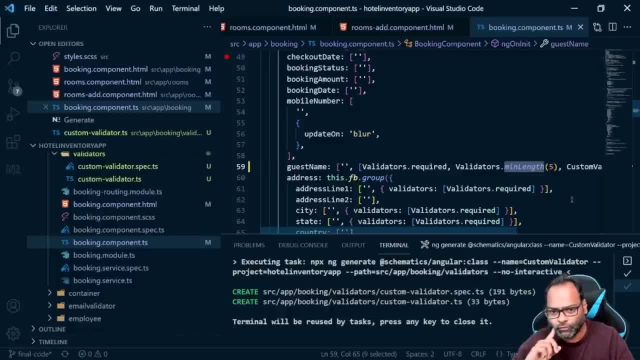 try to write a similar validator and what we will do is, let's say, in case we want to restrict the special characters in guest name- i mean, of course it's not possible, guest name should not contain special characters- but in case someone enters it right, or let's say mobile number. so in case someone enters anything apart from plus, 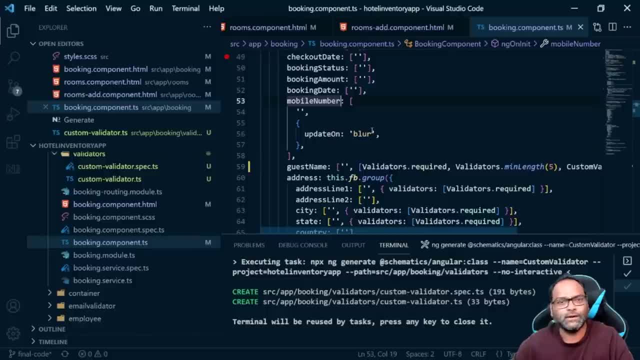 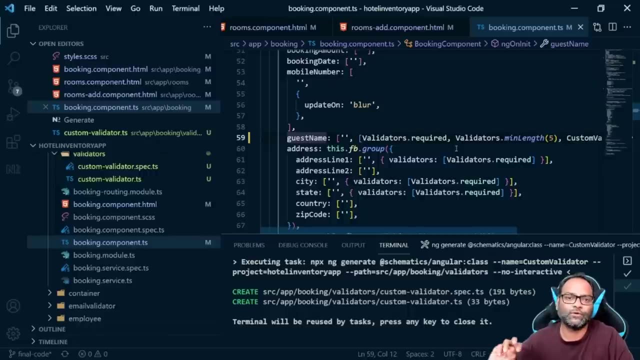 like that: i, i let's. let's not take that scenario. but because it should be number, i mean we can go ahead and directly use the pattern, uh, so it doesn't make sense. but yeah, let's see, uh, guest name, let's take guest name and what we want to do is: we want. 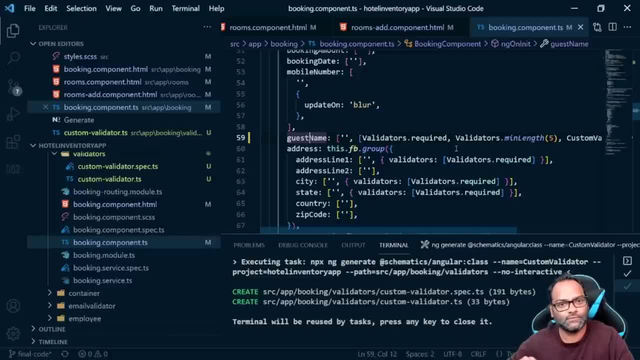 to pass, uh, some characters which should not be allowed. so it's, it happens, right? so perfect scenario for your passwords. let's say you have a password control and you want to- uh, you don't want to allow some specific, uh, special characters and you want to rewrite the custom validator for that. 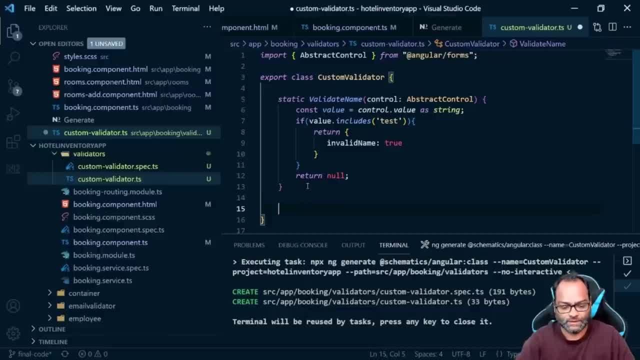 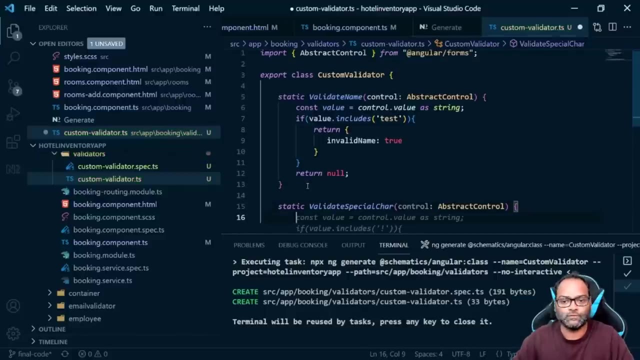 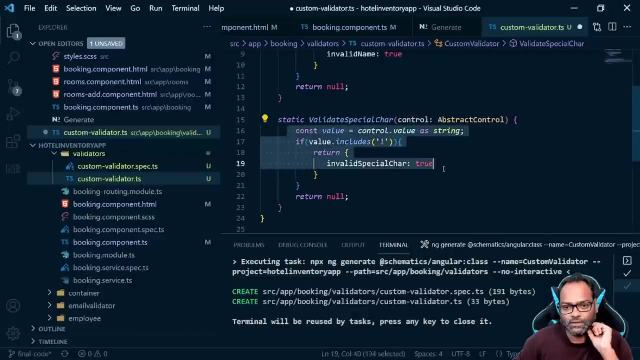 so what we can do is let's write one and say: this is static, special care, right? so we are saying, okay, uh, let's see. so we are saying okay, uh, this value. but you might be wondering right now it seems similar to this: so what we are missing? so let 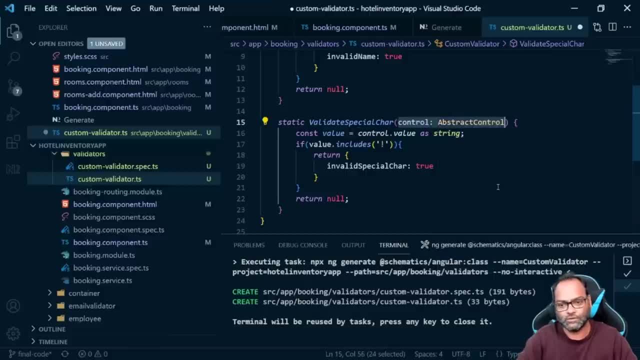 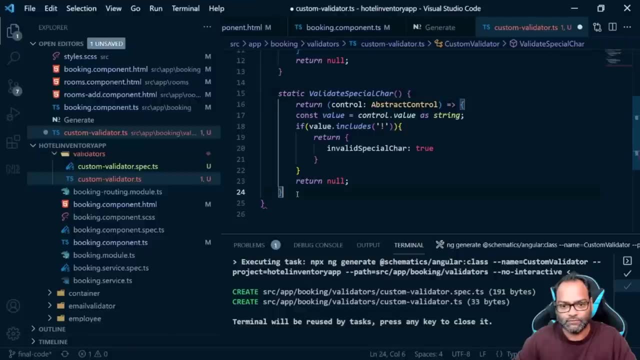 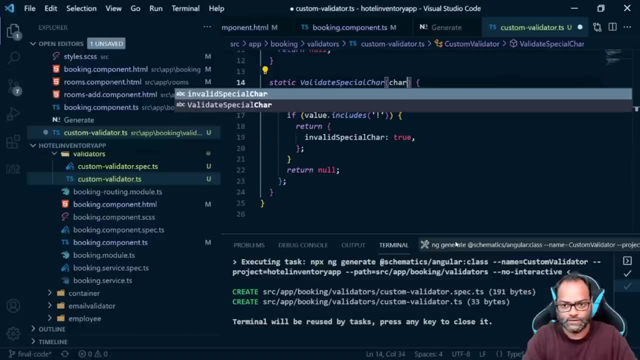 me just show you what we are missing. so, rather than passing the subset control here, this we will change. uh, we will return control like this and here we will, and we will pass a character here. so it's okay, this is character, which is type of string, and we will check for this character if this character is available. 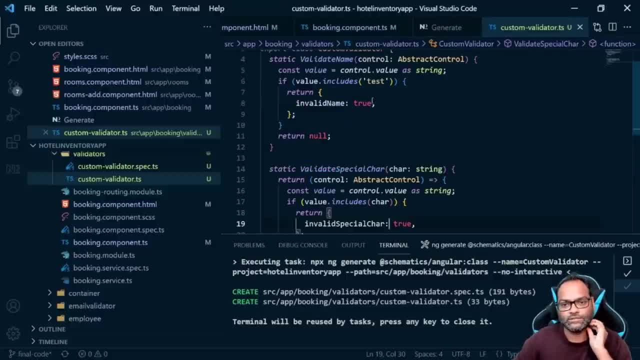 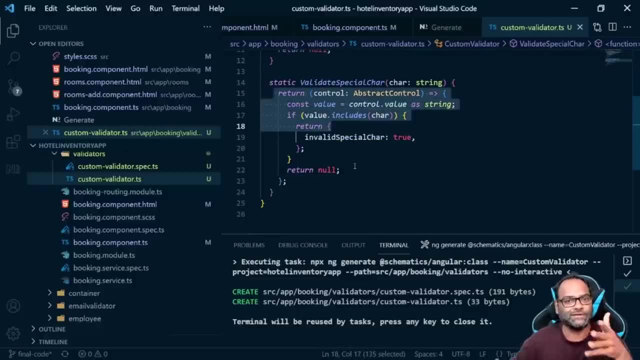 okay. so let's uh see what we are doing. so, rather, actually, we are going to return control and we will pass a character here, so let's say a character passing the object directly. we are returning the function, so it's a function inside a function, right? so this is the main function which will take the parameter and then it will return a. 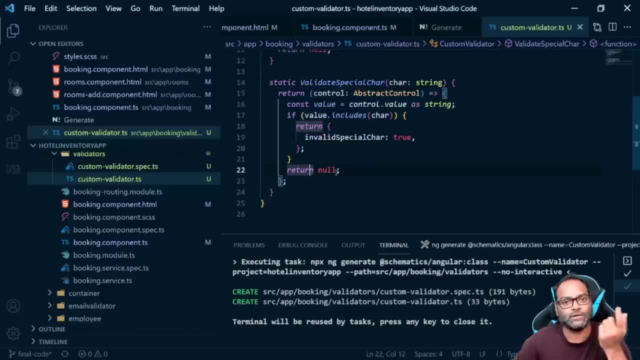 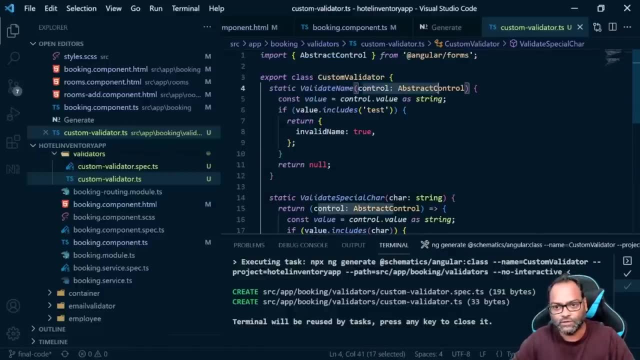 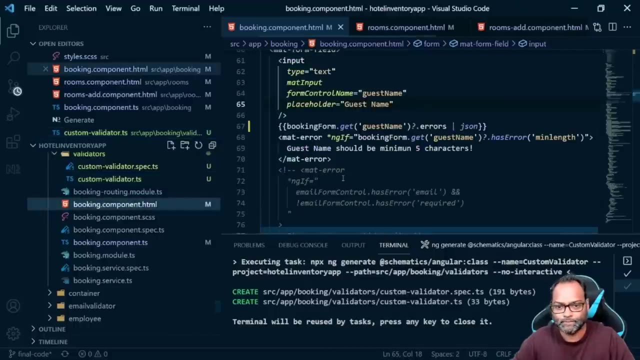 function which will return either invalid special character or return null, and to use this, there's only small syntax change, if you see. so, rather than passing this control here, we are just. we just moved it inside here, so let's try to use this and we'll apply it on the same guest name. 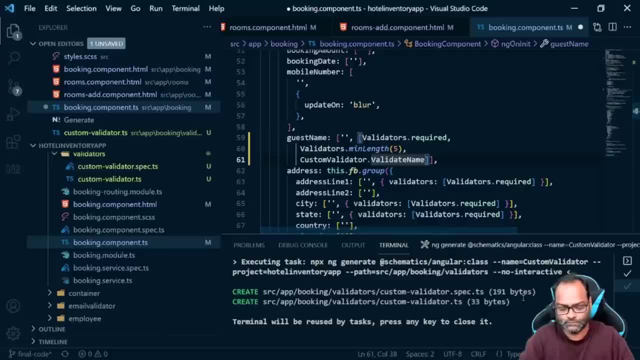 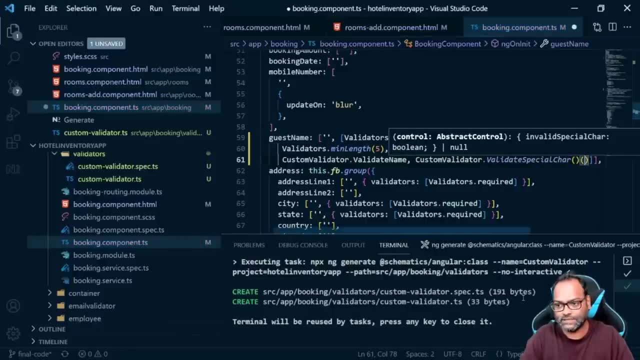 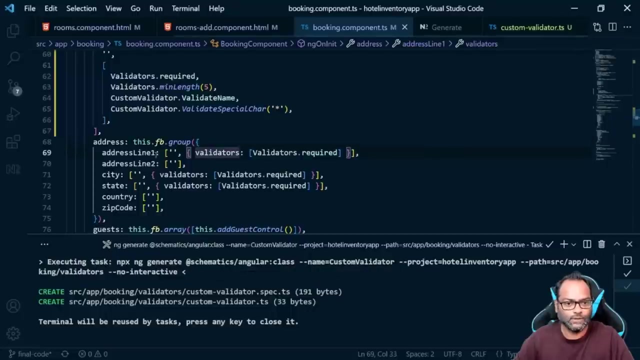 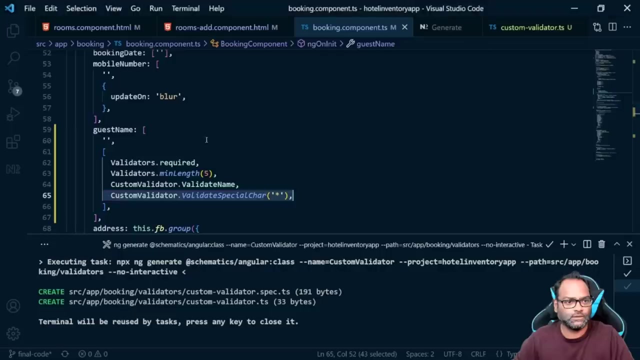 you can say: custom validator, dot validate special care. let's say we are not supposed to use stuff, okay, so we'll pass start. and if it the same handle of of val, so we have that one here, so we do this. okay, let's call the. if so, if this, uh, if someone enters a star into this particular guest name. 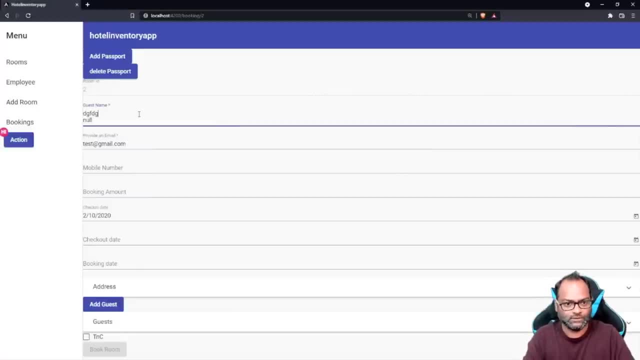 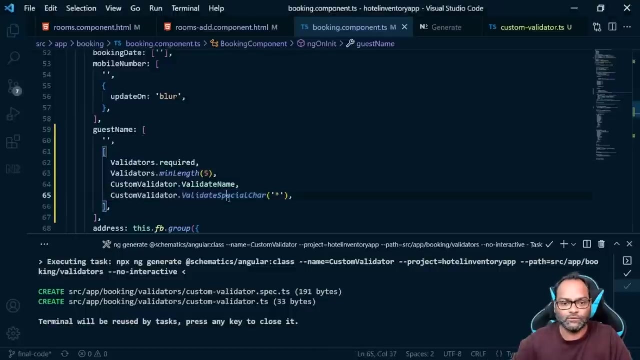 it will be invalid name. so let's enter to do that. so we are entering the right name and a valid name, but we entered a star, so it says: okay, this is the invalid special character, so you should not use star. so this is how you can do that. you can, of course, implement. 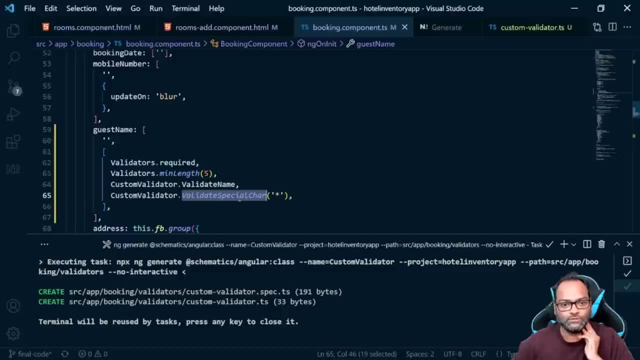 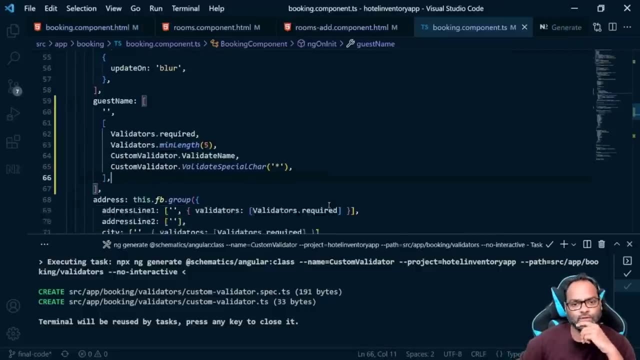 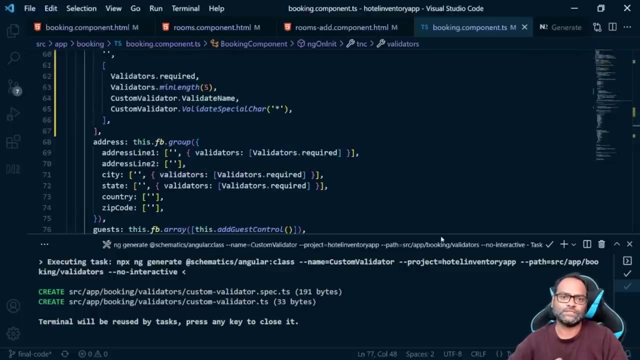 what you want because of the current. so now we're ready to enable this one. we open the your own, whatever you want to pass, i mean. so whatever character you want to pass. now, third scenario which we will talk about is for form. so where this type of validation is, 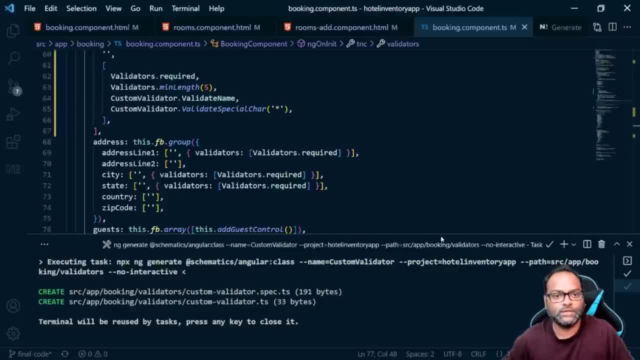 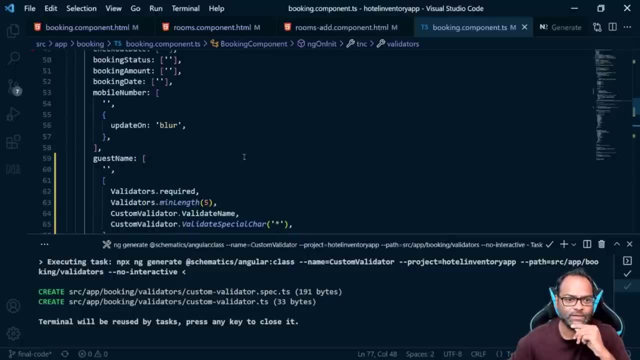 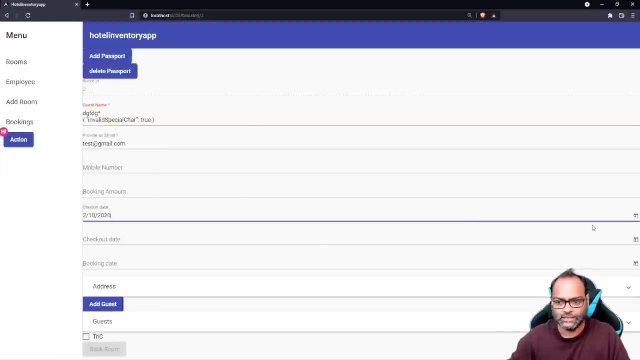 sorry where this type of validation will source. so let's say you have two controls right which you want to validate, for example password, confirm password. here also we have an example. we have this check-in date and checkout date. right now i can just go ahead and say that my check-in date is: 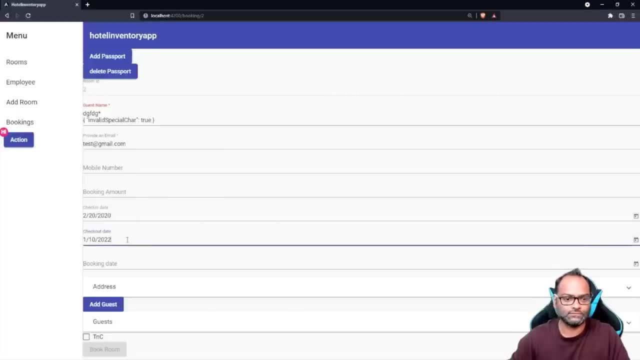 20th and checkout date is 10th, which is not possible, right? so what in case? we want to write a validator which validates this? which validates, okay, this check-in date cannot be greater than checkout date, right? so let's try to write a validator for this. how we can do it? let's go back to our validator. 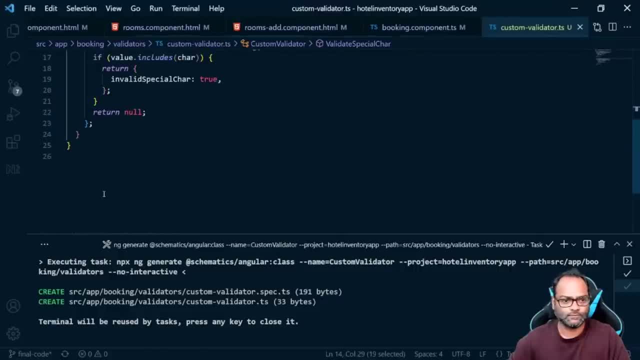 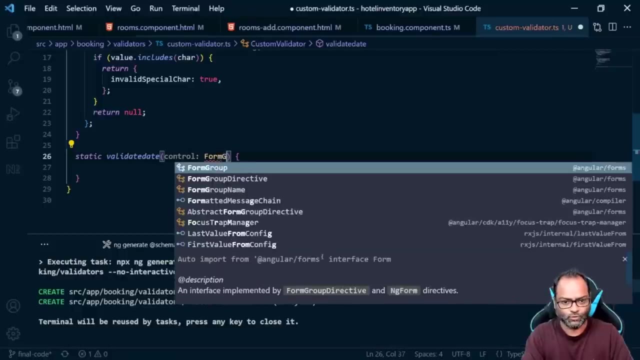 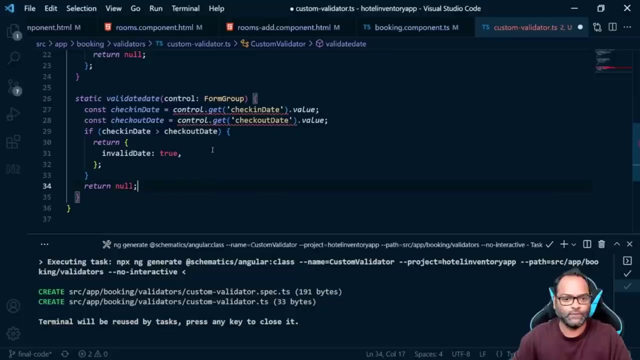 class. so let's say this is static. we'll say validate date, but rather than actually passing abstract control right now, i know that this is this is a form group and here we will get the values for both. so we'll say: okay, give me the control called check-in date and why this is giving an issue. 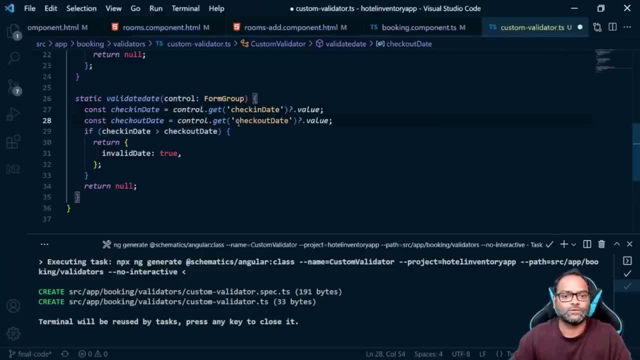 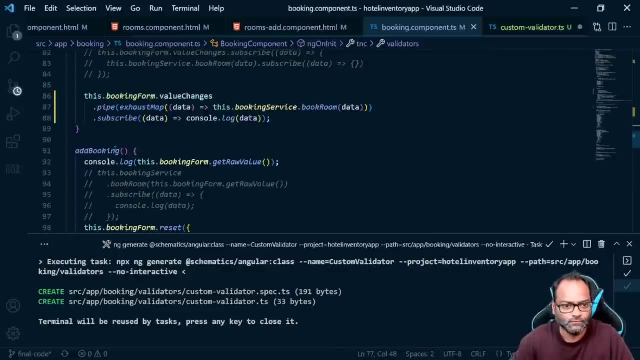 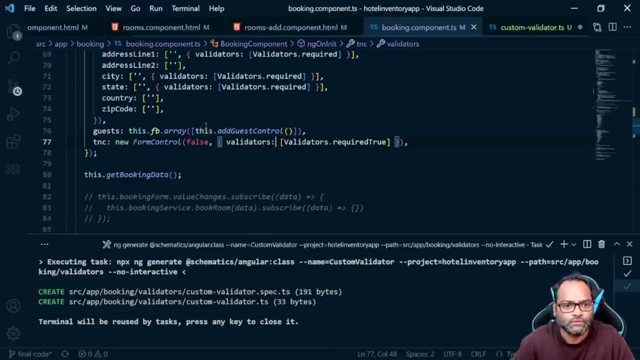 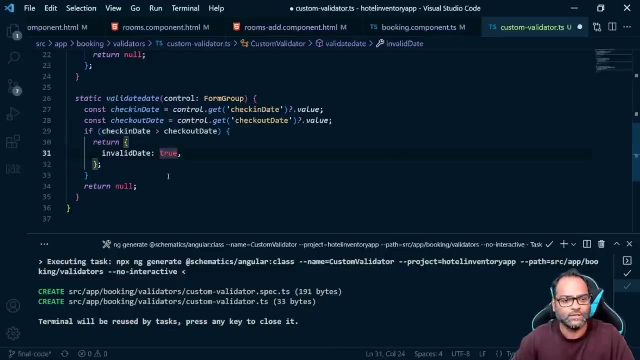 ah, okay. so uh, we, i'm saying, give me the value of check-in date and checkout date. let's verify the names. i mean because this, this object, should object name should match. so we have check in date, check out date. d is capital in both the cases. yeah, looks fine, but let's put the logic to actually. 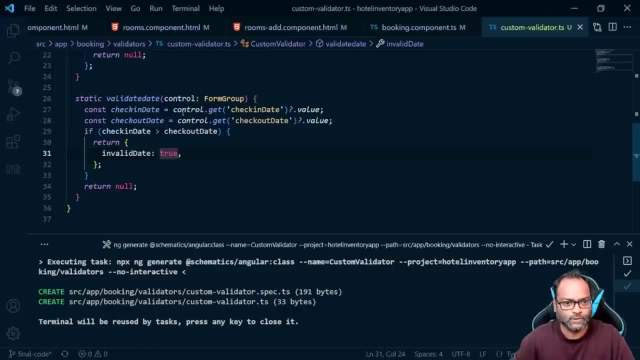 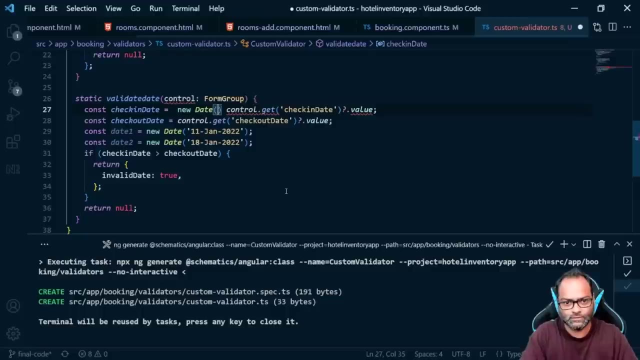 calculate the date. so i'll say: this is you, i'm just typecasting it to date. so we have this one and this is, and this is new date, and we'll take difference between two dates. okay, first we need the time. okay, first we need the time. 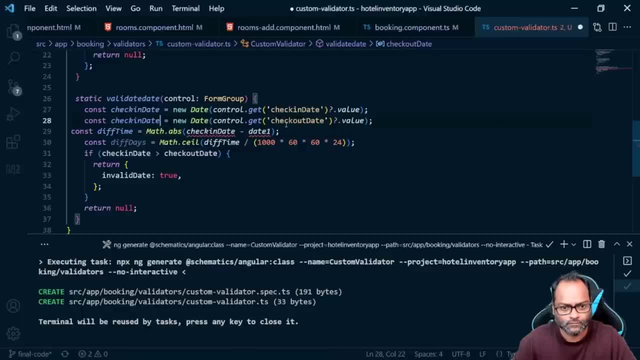 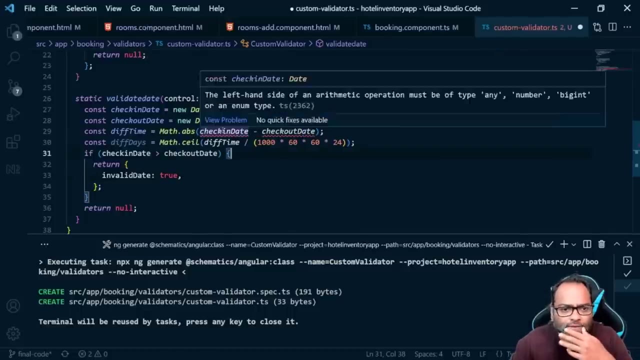 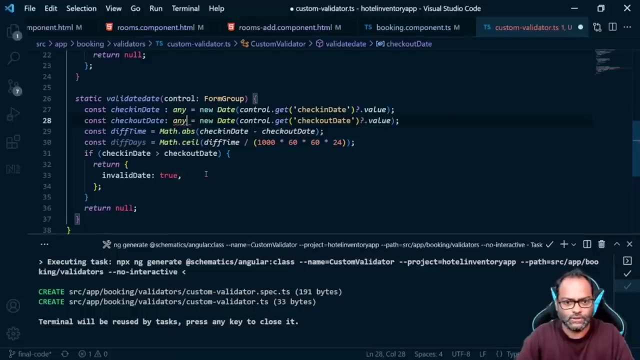 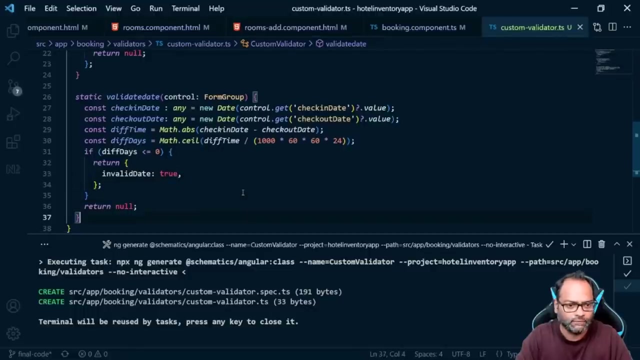 Check-in date, checkout date. Let me just typecast it to any right now so we can see: the stiffcase is less than equals to zero. I'll say this is invalid date and otherwise let's verify this logic, right? So what we will do is we will just do console dot log. 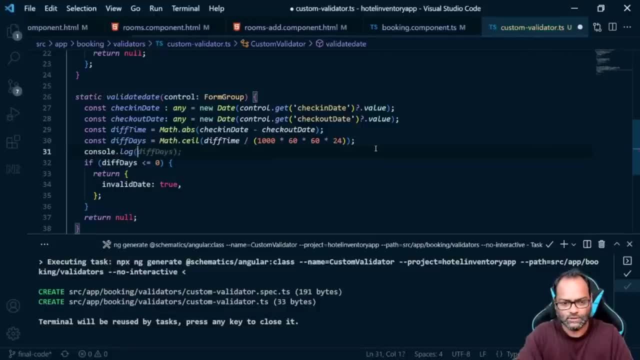 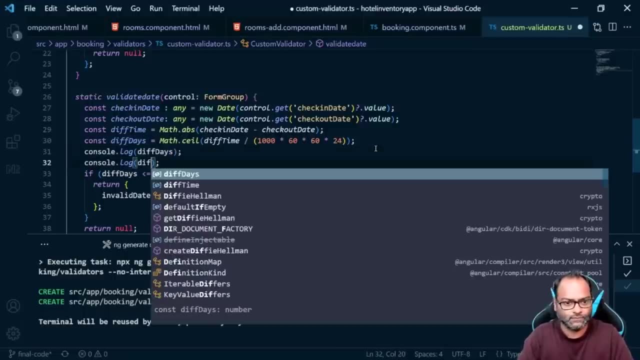 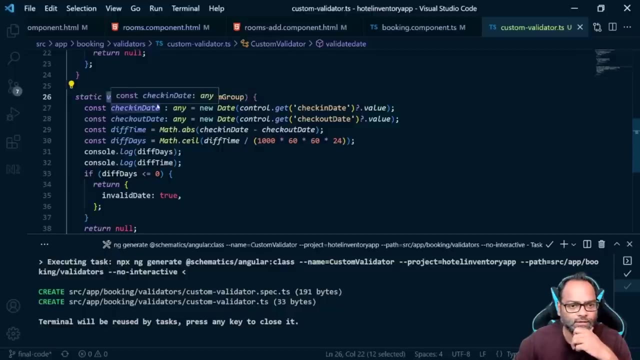 For all the values, to see if this is what we are expecting- div days, div time- and let's use it. So what we have done is we wrote a validate date function which takes form group and we are checking, getting the two values- check-in date and checkout date- from this and then 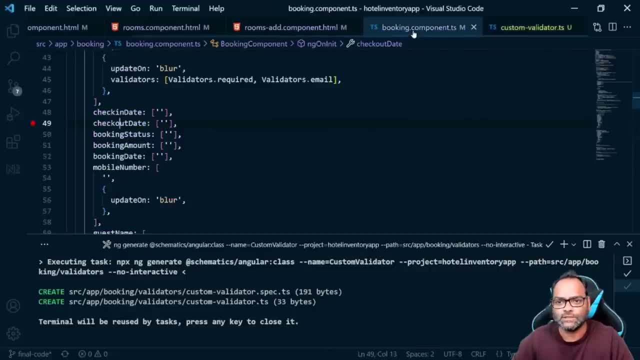 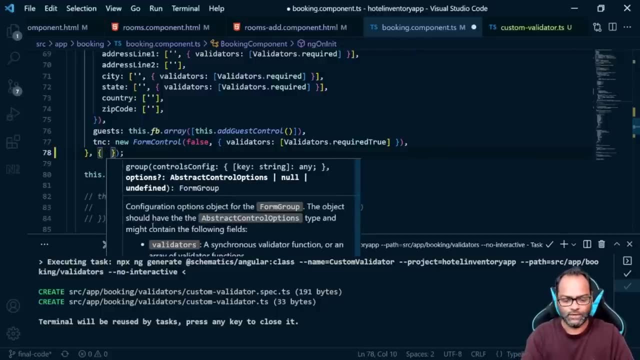 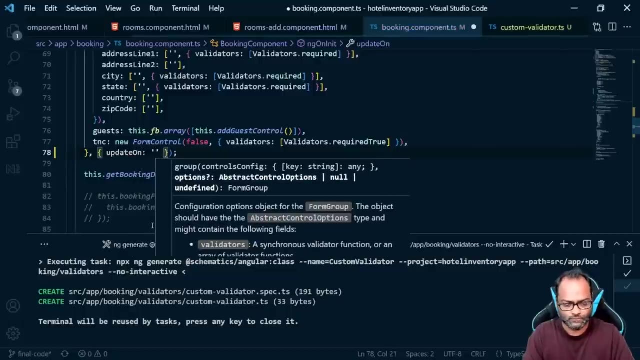 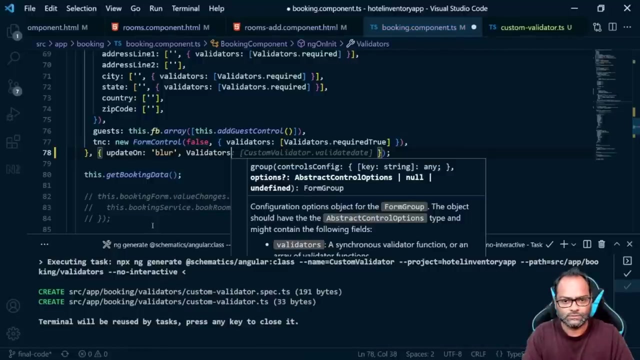 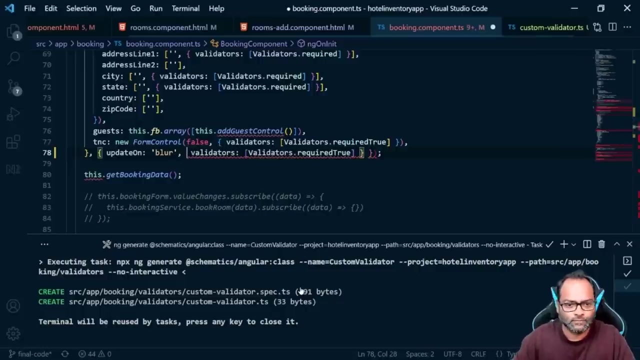 we are calculating the difference. Let's go ahead and apply this on Booking Component: dot DS, and what I want to do is I want to call this particular method runs. my update on value is blur- And I want to call validators And which is custom validator, dot validate date. 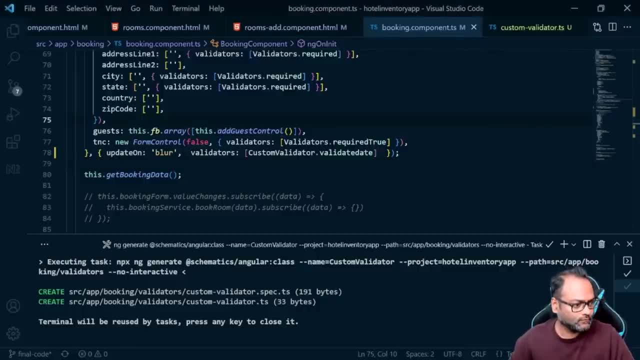 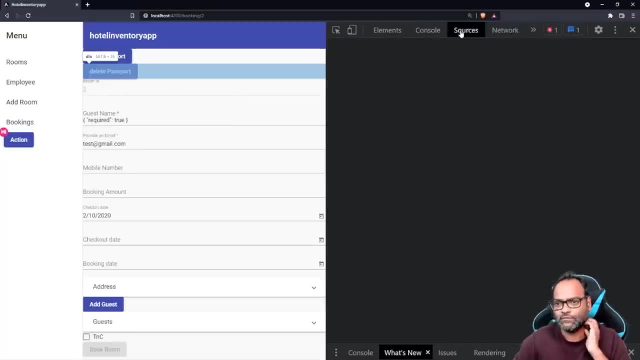 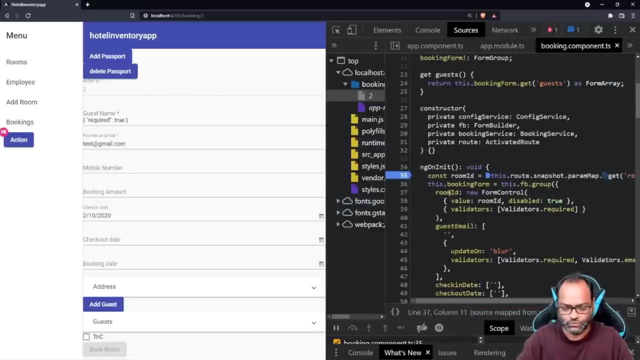 Okay, let's inspect and we'll add a breakpoint so we can see what is the value which we are getting right now. So I can say here also: to search a file, you can still let me show you some shortcut as well. You can just press control P, control P on your keyboard and then you can just start entering. 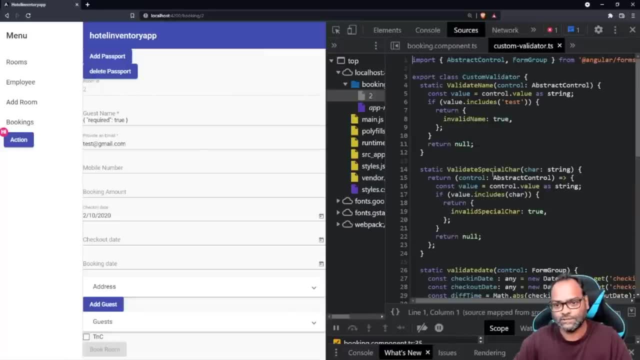 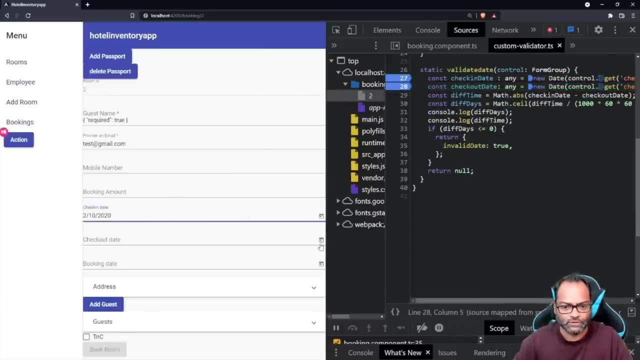 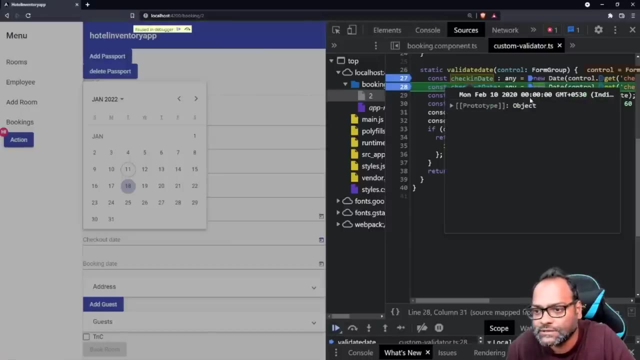 the file name. So I need custom validator or DS, And let's add some validation. sorry breakpoints here. Let's choose chicken date, which is already there. Let's choose checkout date and let's see, So we have chicken date as this Monday, February 20th 2020.. 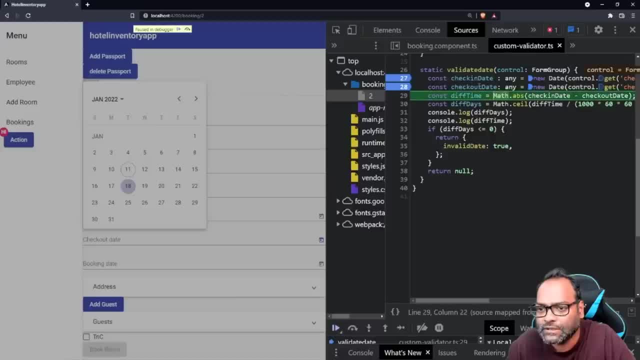 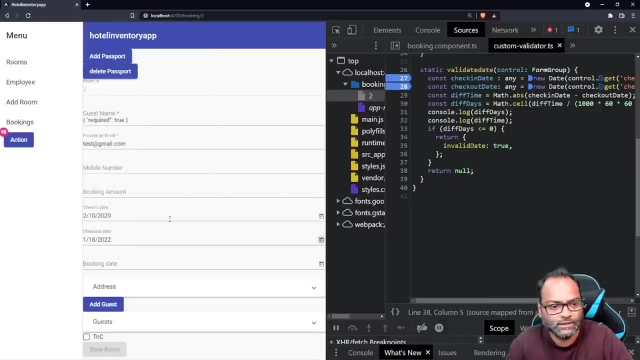 And then we have checkout date, Which is Right now, Jan Jan 18th. let's say the difference seven and eight days, And if if days is less than equals to zero, then invalid, otherwise valid. So right now the form is valid. 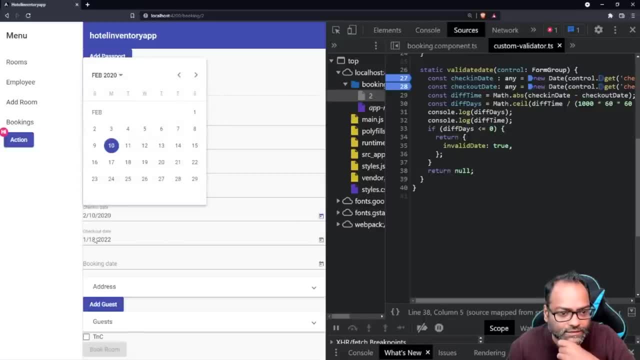 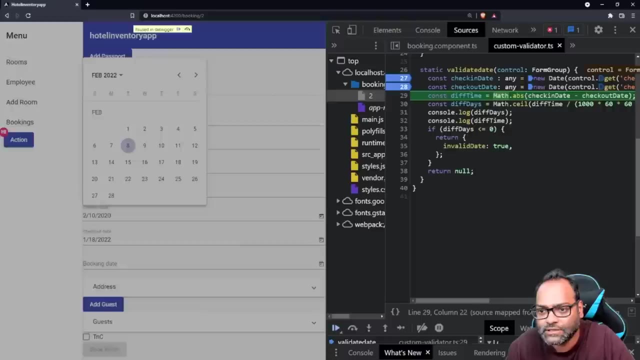 Let's provide a date. So this is 18th, Right? So let's select Check in date after January. So let's see now. So Check in date, check out date, and then dip days should be minus right now. 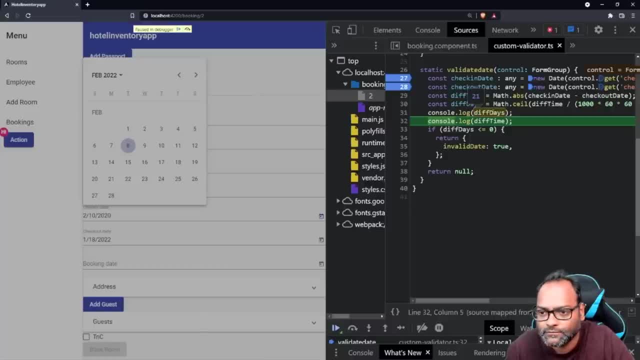 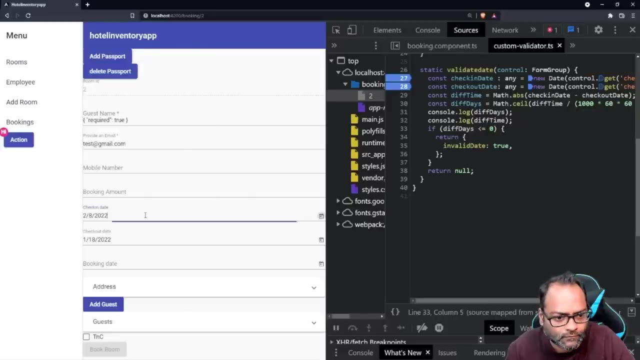 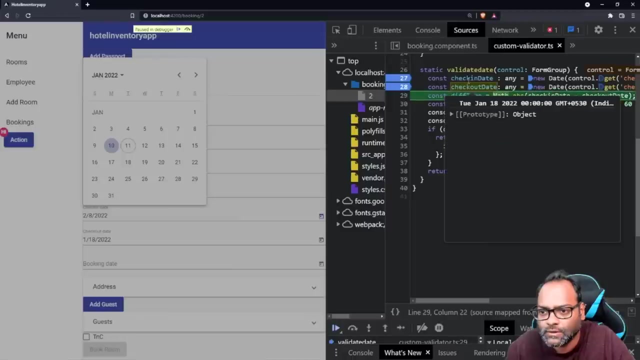 So OK, somehow it is 21.. How come Checking date minus checkout date? OK, let's try to select 10th, So Jan 10th, Jan 18th, Because we are doing absolute. That's the. 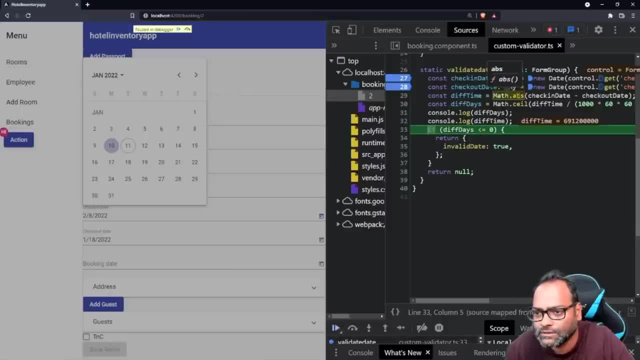 That's why it is. That's why it is. If you want to, If you want to see the date, you can see the date that you want to see the date, And so So that's it. So that's it. 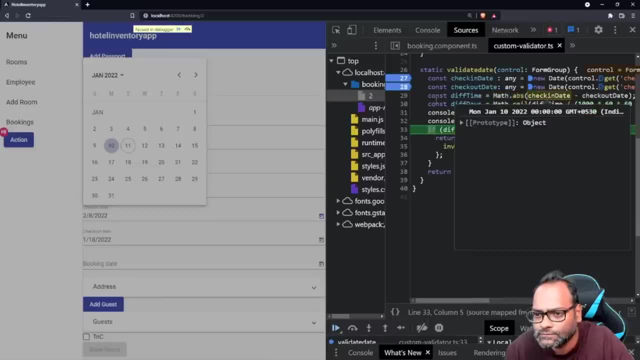 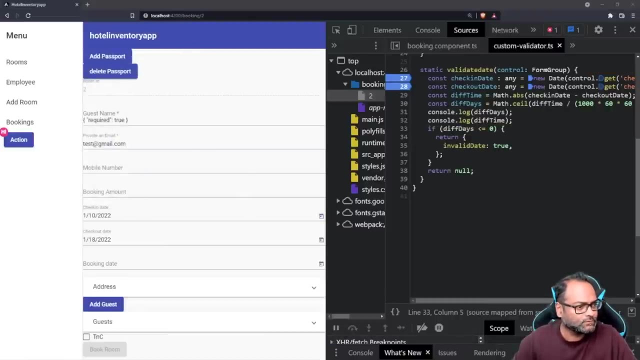 So that's it. So I'm going to, I'm going to, I'm going to. So let's start, I'm going to. okay, probably something wrong, let's see. so we were right. i think this, uh, it is happening because of this math dot. absolute, let's go. 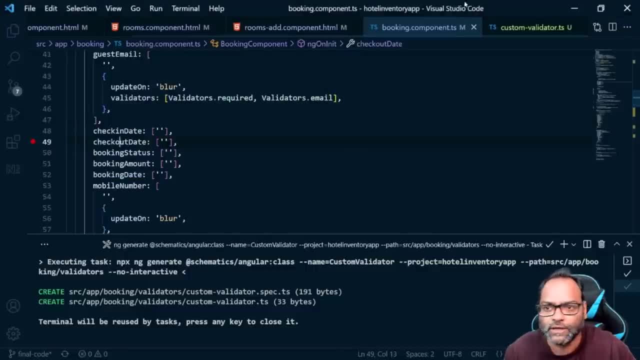 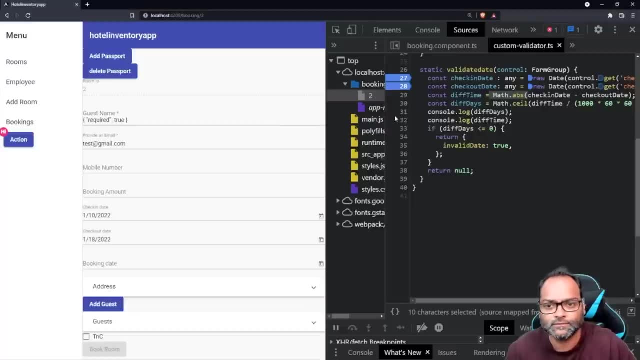 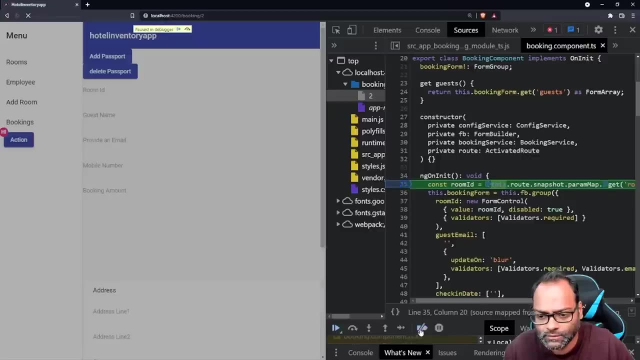 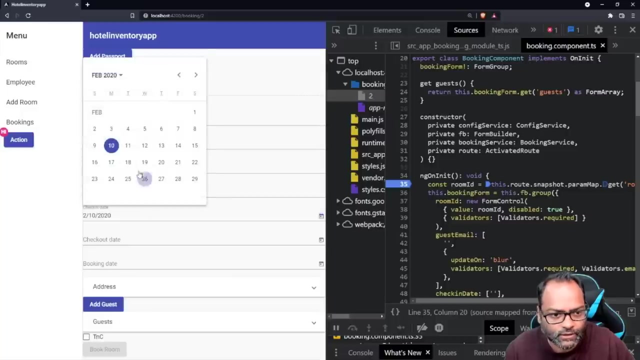 ahead and remove this mat dot absolute because it is. it is returning us positive value and in case we need the diff in minus, we should. let's try this out and just disable and run it and let's enable. uh, now, let's provide a date, so we'll just 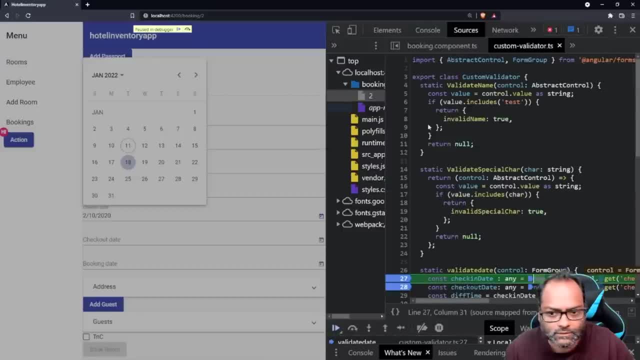 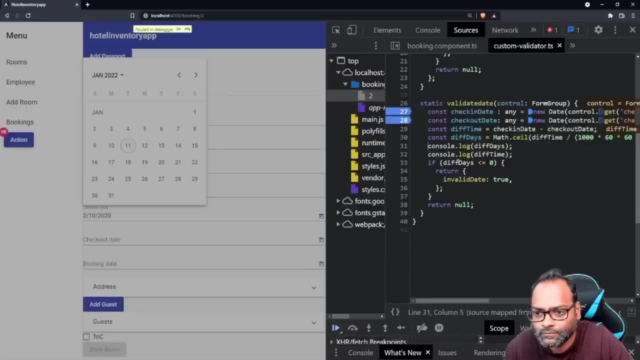 select 2020 jan 18th. so, uh, right now. okay, this is not a number, that's, that's okay, and let's select a previous date and day days is 18th and 10th. okay, so it should be checkout date minus check-in date, if i'm 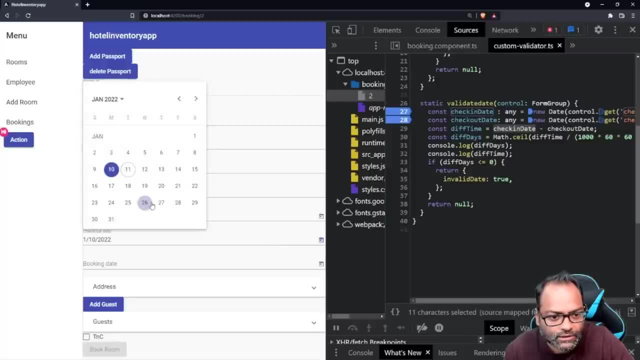 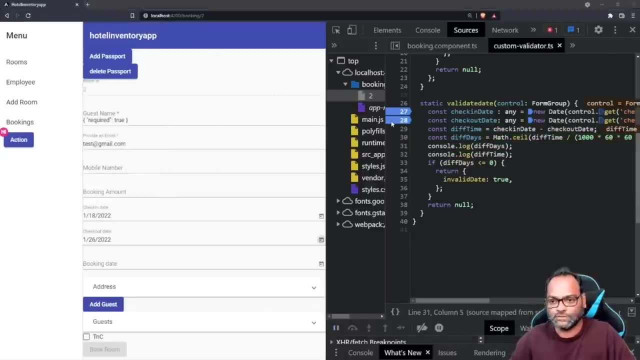 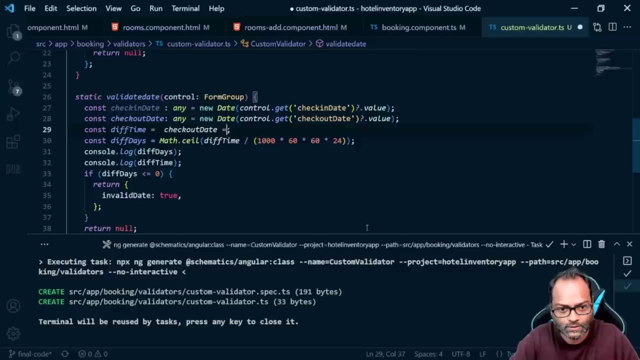 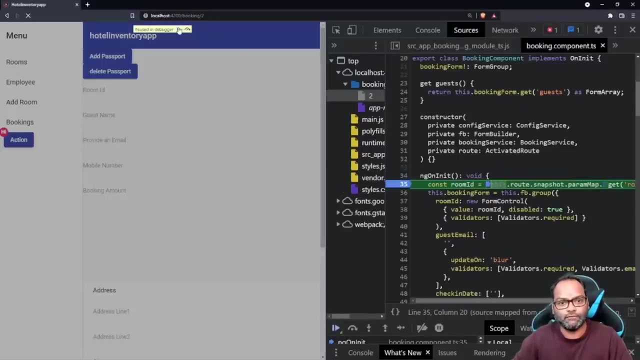 not wrong, let's try this out. so if i put this date on 26th, i think we should now get a minus value. yeah, so, yeah. so we just need to now change the position so i can say check out date minus check-in date and we are through. so now we have added a validator which validates to date, right, and 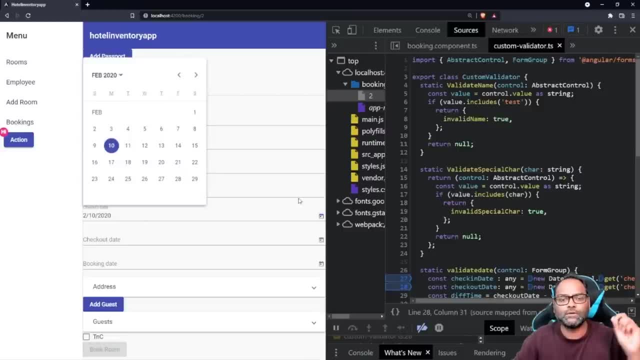 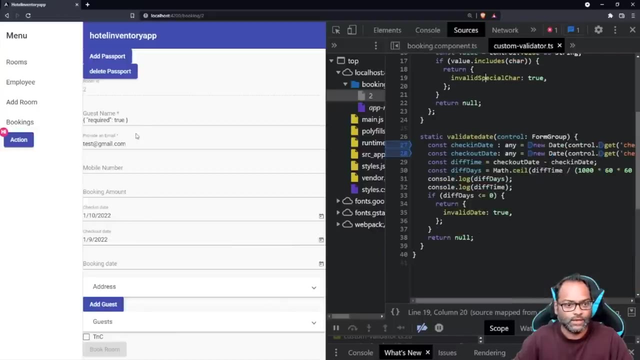 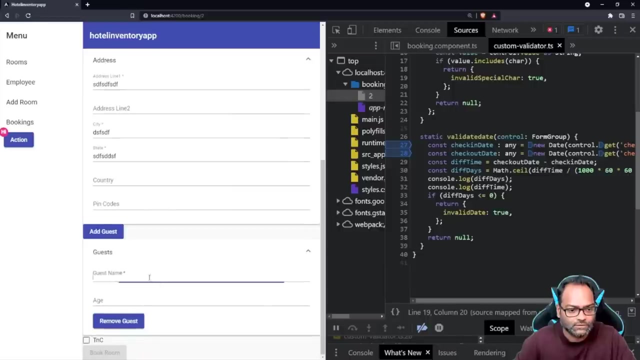 this is something which you can also take and apply to password and confirm password. so let's supply jane 10th and so, And if I try to check out early and let's apply, give all the values, valid values, mobile number. let's see, just want to give the valid values or required values, right. 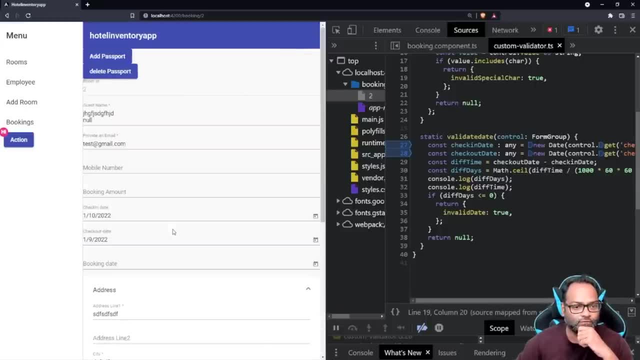 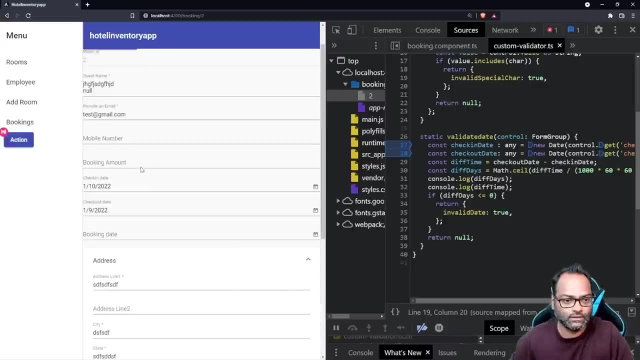 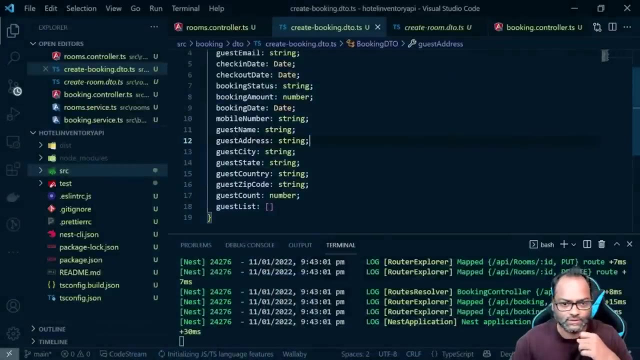 So, even though we have provided all the valid values for required fields, there is still a problem with the form validation because the date condition is not satisfied. We cannot check in. sorry, check out early. So let's go ahead and see this first. 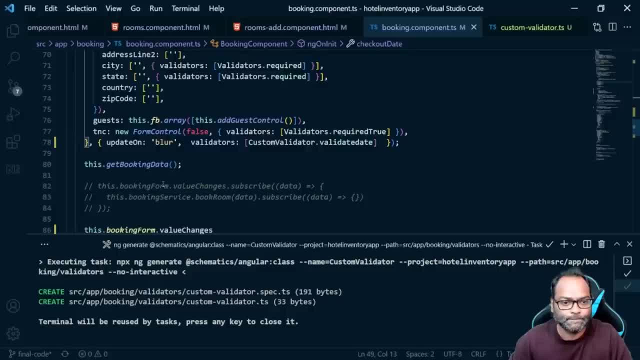 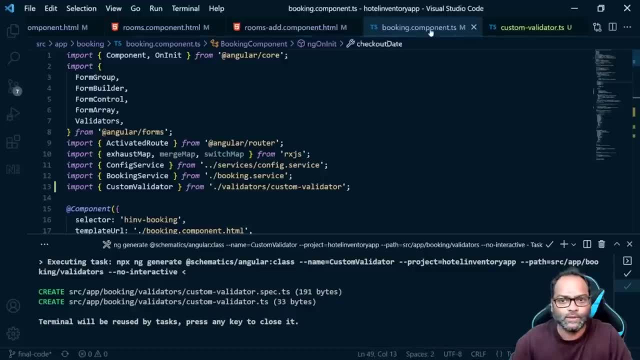 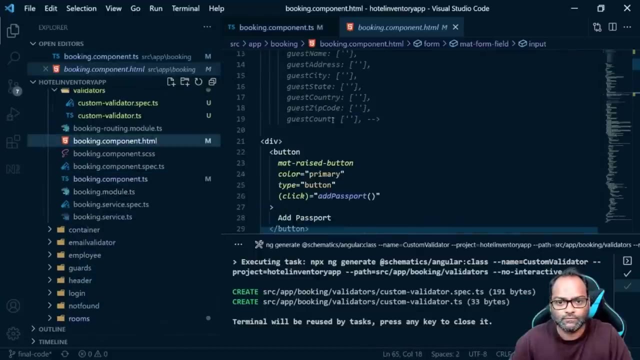 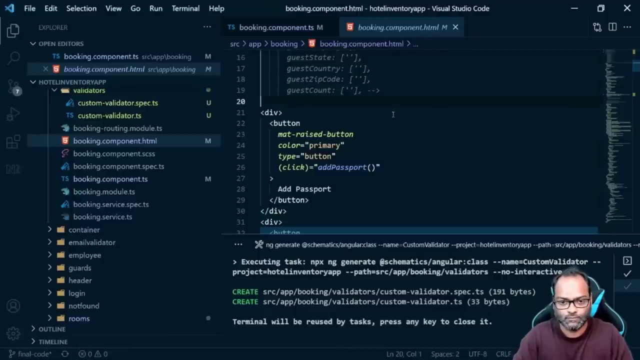 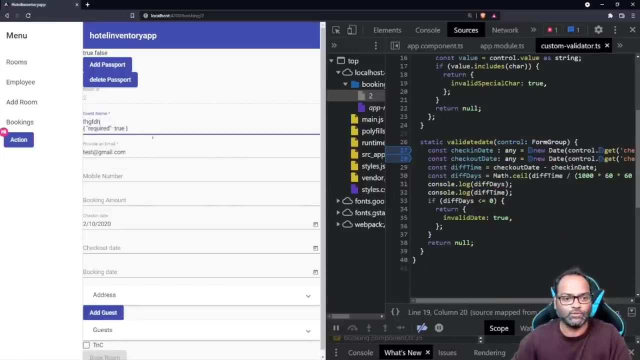 So here I can apply: Okay, okay, okay, Let me just close, So you can right click here and say: close others, Booking form Dot Invalid And we will do one thing. So right now it's really hard to figure out right where the problem is, because 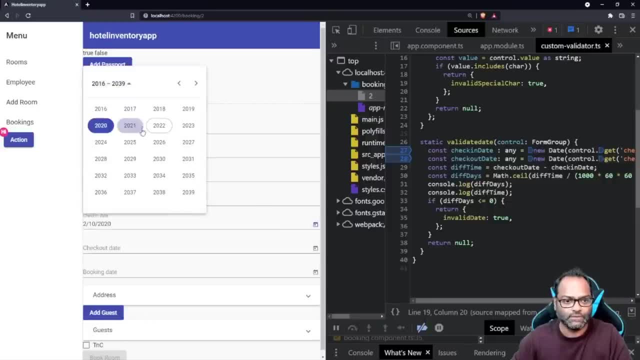 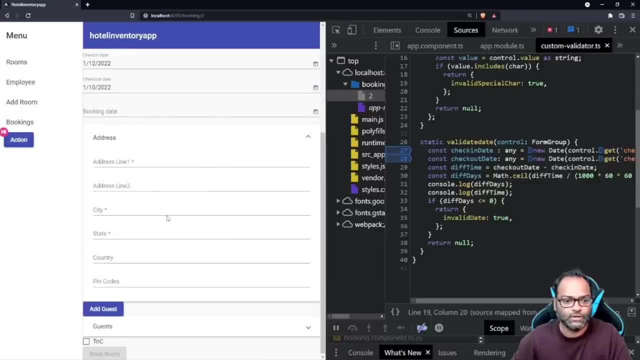 we are saying, Okay, this date does not match, but we are not displaying any errors. So it will be really confusing for our users to figure out the actual error. So what we can do, of course we can add a control level validation. 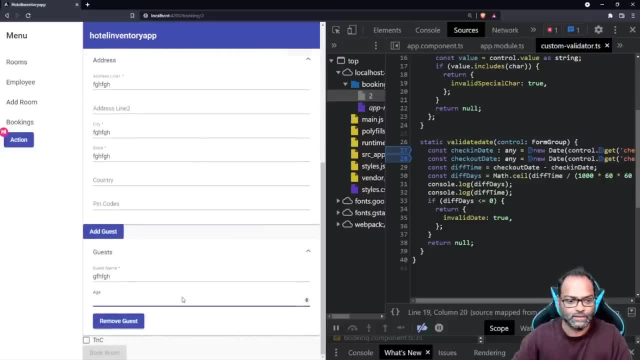 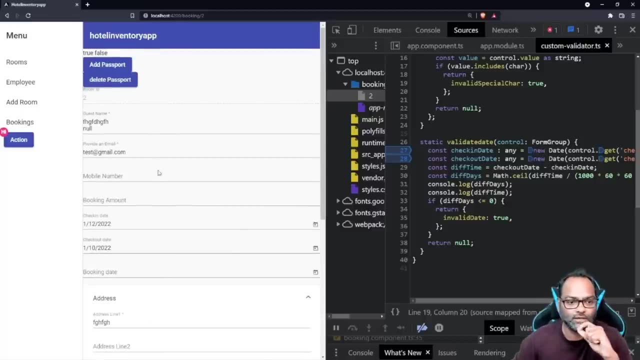 So let's do that. Let's try to see how we can apply this to a control level. I mean how we can actually apply this error to a control level property. right now, This error is actually available on Form. It's not available on the control. 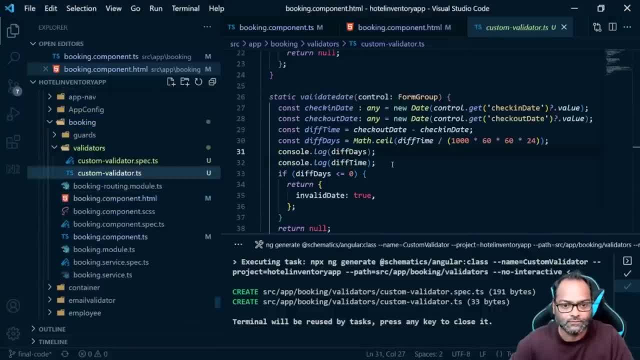 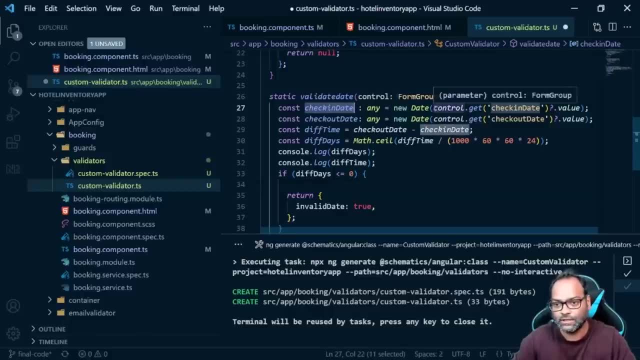 So what we will do is we will add: Yeah, so we can do something like this, So we already have access to the control. So, if you see, this is a control checking date and check out date. So here we can add something like this: 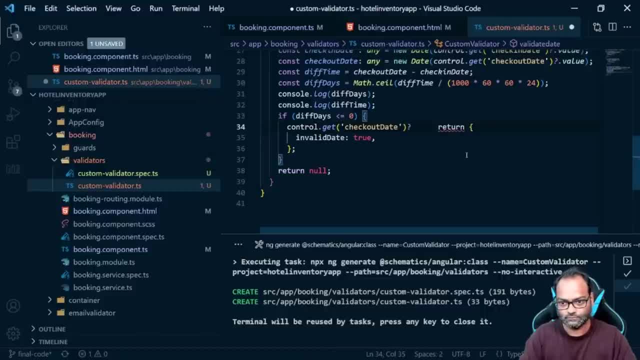 Uh, get Dot Set error And we can see: uh, invalid date, true, and of course it can be null. So just put it here and now. this error will be added to your control. Let's go ahead and try to figure out if it's true. 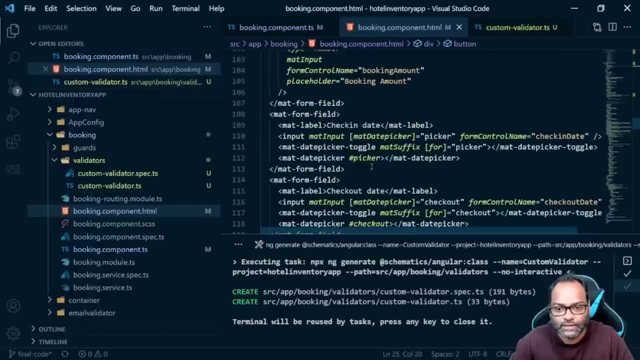 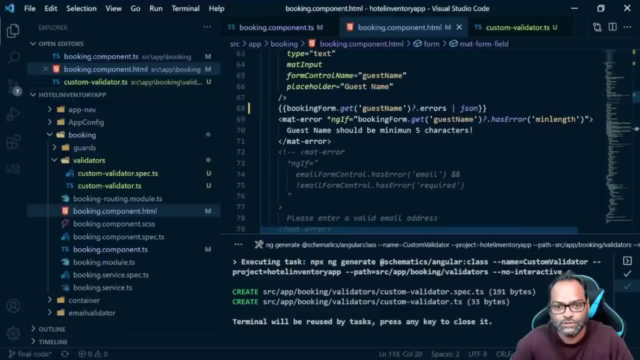 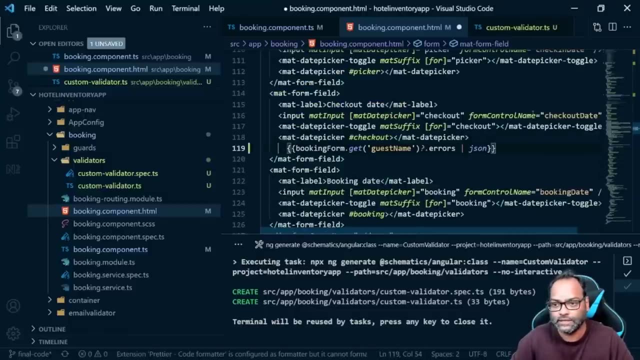 So we will go to check out date. checking date- check out date. This is our checkout date and we will use the same approach to print the Booking date check out date. here it is. So we'll take Check out date. dot errors- check out date. 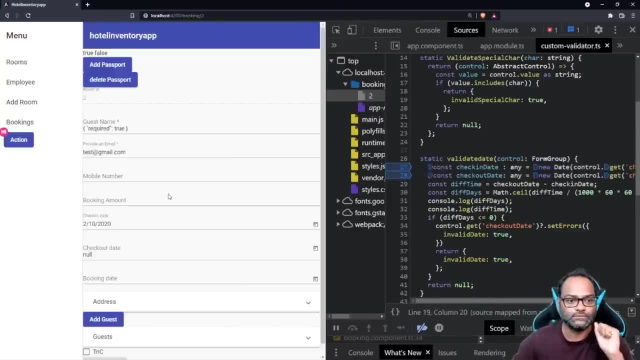 And let's see, let's see if this particular control is applied to the uh checkout date or not. So let's select a date: 2020 Jan, and I'll say 18th, and check out date is 10th. 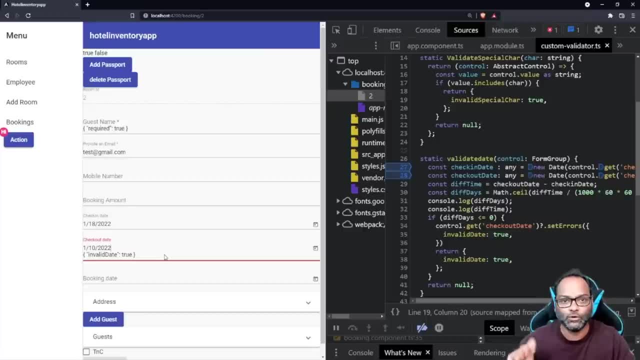 So you can see: uh, it has an invalid date error, which is applied to the control right now. So this is how you can actually also show meaningful messages to your end user. So They know, okay, what we are doing wrong. 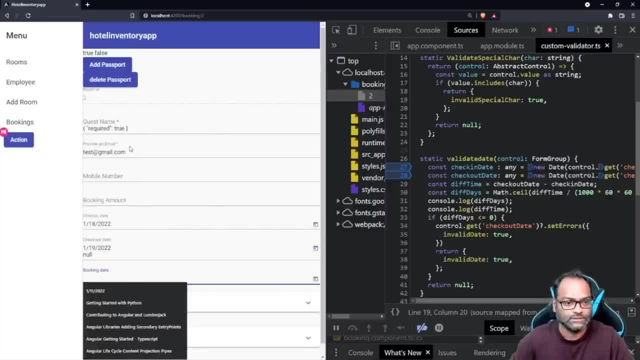 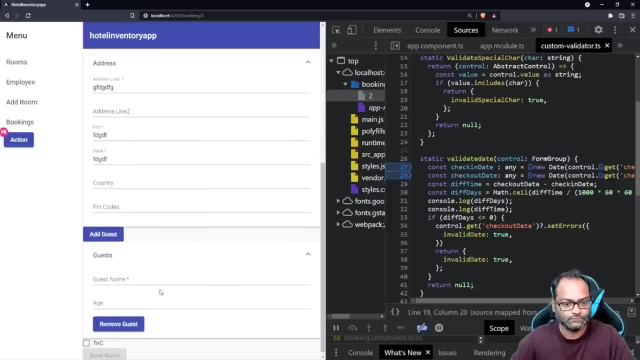 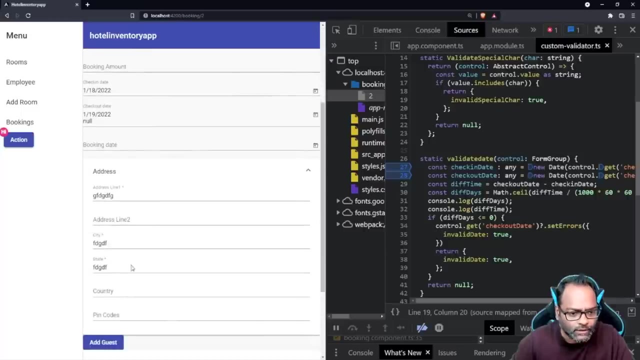 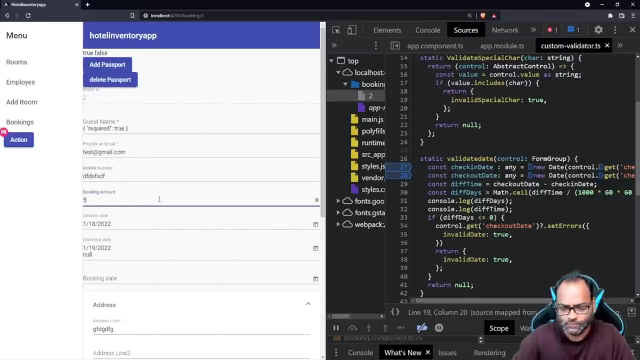 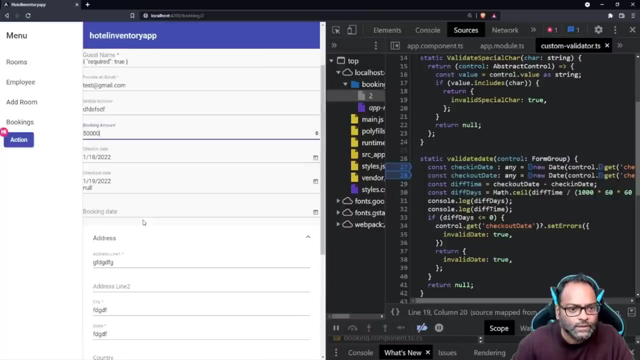 Now let's go ahead and print, uh, fill in all the valid properties and let's try to submit this form and DNC, And it looks like there is one more validation error which is not satisfied. Which one? Okay, Which, which, which? which property is that guest name? 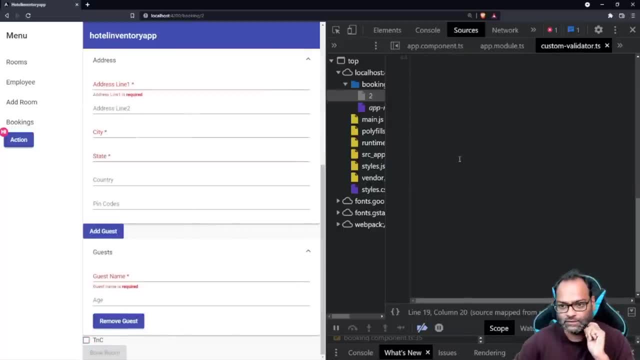 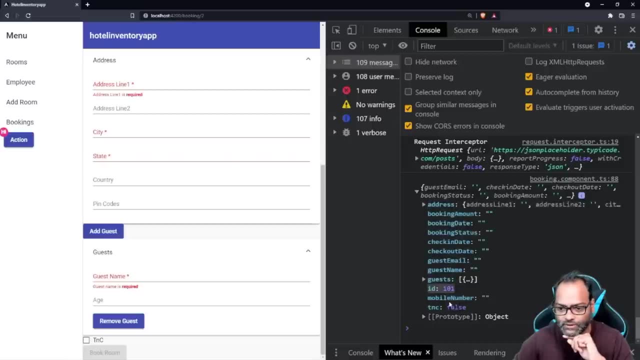 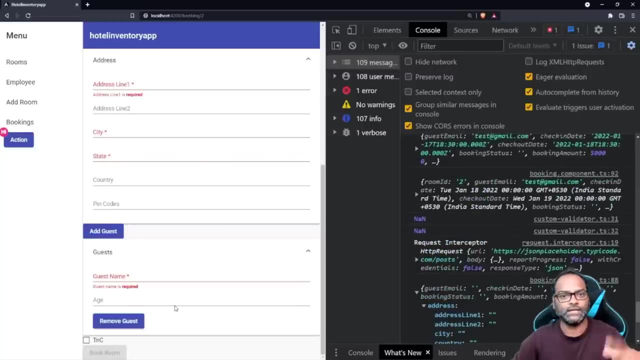 And here it is, So now this book room is valid. We submitted it. Let's see, And this is your guest email data, which is available here. ID is one zero one mobile, And So I remember, right now we are actually sending this data to a dummy API, right? 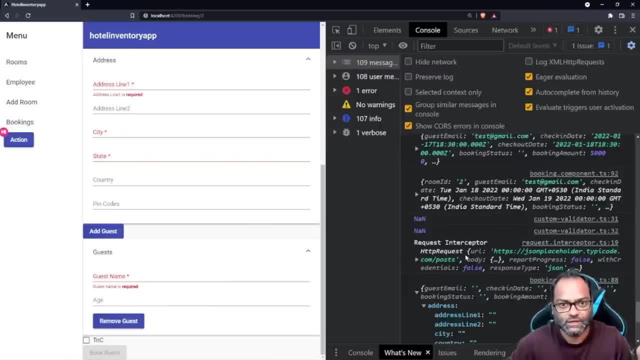 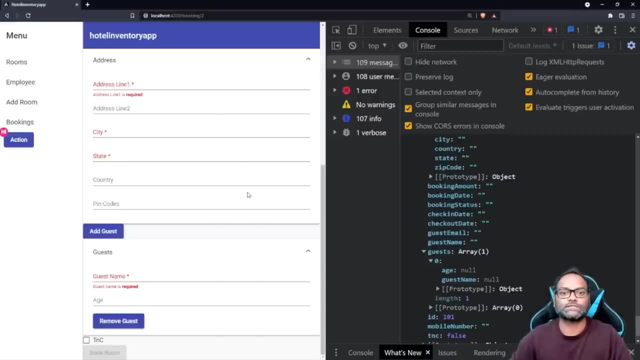 So which we which we wrote, uh, I mean, which we, uh, uh, took it from Jason placeholder, So we are just sending this data back to. that's it And this is it. So, uh, this is how you can add custom validator to your reactive form. 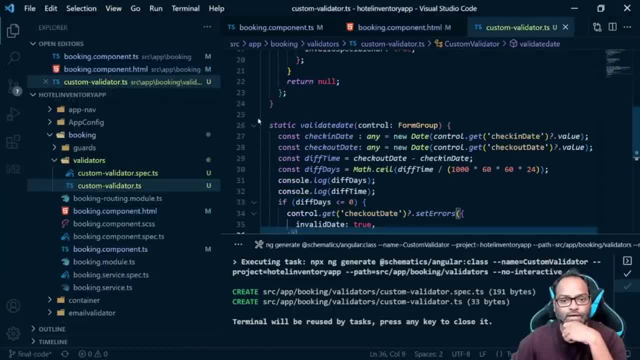 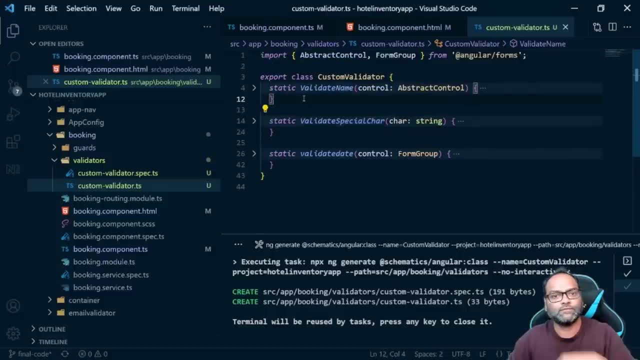 We covered all the scenarios, all the scenarios which we can think of and which is useful in case you are writing the validators for your application. So, uh, this is it from the customer, Where the setup is, because we are sending it to a product. 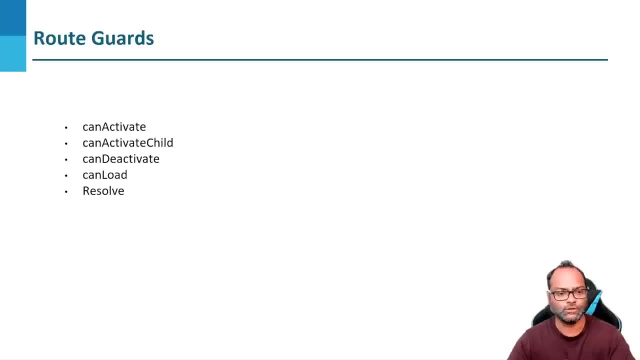 And this is all what we have done. Certain, uh, talk about one route guards which we had left. We actually have to lift a. we will come to the Zogar, but let's see, uh, let's talk about candy activate. 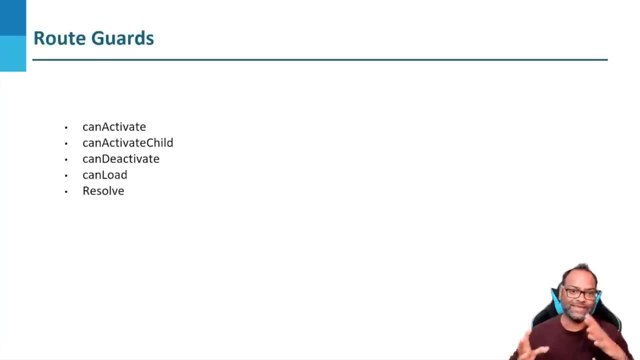 The end. the activate guard is something where we are saying that, okay, now you have entered the route, but can you exit the route? So we have Trying to. user is actually authorized to exit the route, right. so here example can be, let's say you: 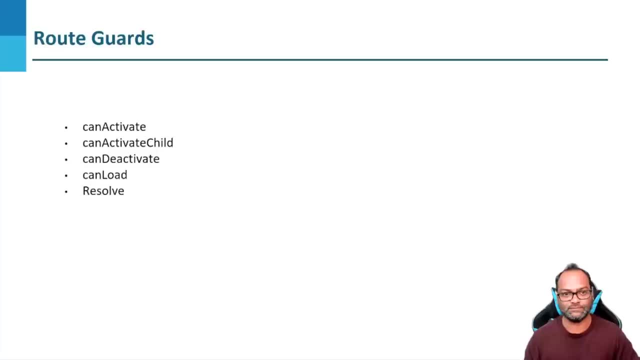 entered into theater but can you exit the theater? i mean, probably you need some authentication to exit, so you are blocked until endless, let's say, movie finishes or you have interval. so to generate or to have a real-time scenario here, what we will do is we will create, we already 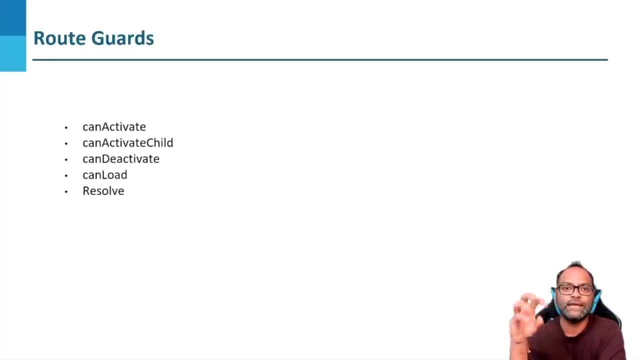 have a booking form. so what we will do is, in case there is some information, or, let's say, our form is in dirty state, it means, as a user, i came and i made some changes into my form and if i try to exit, we should display some message, let's say saying: 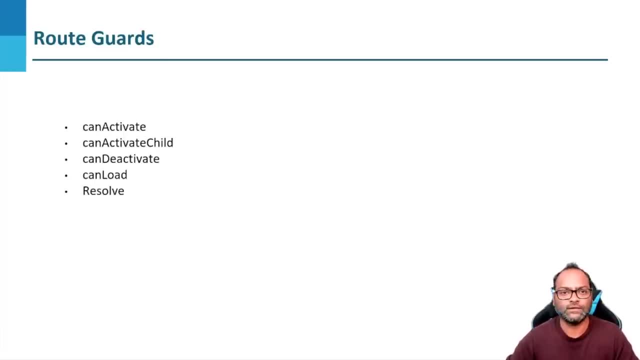 you are not authorized to actually, or you have some pending changes, and if i try to exit, we should display some message. let's say saying: and if i try to exit, we should display some message. let's say saying you can display a pop-up saying you have some pending changes. do you really want to exit? 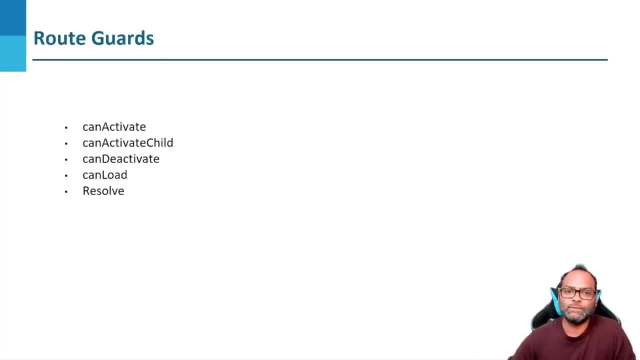 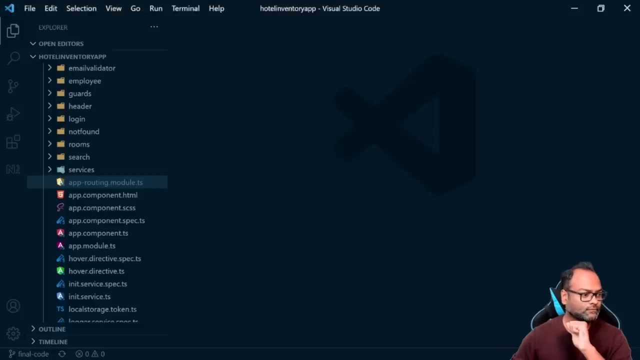 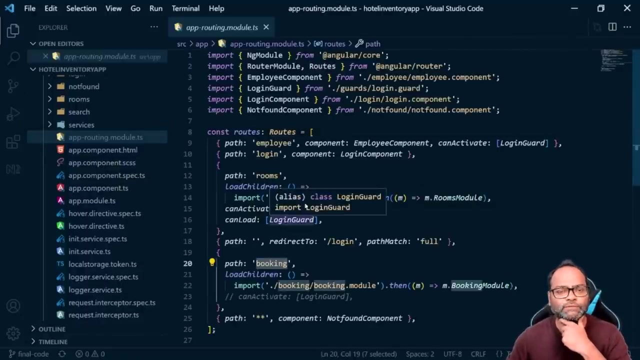 some kind of message, right. so we will be trying to generate the same scenario. so let's see that with candy activate, the one thing is you can do it for a routed component. so if you see, our booking is actually one of the routed component which is available here. 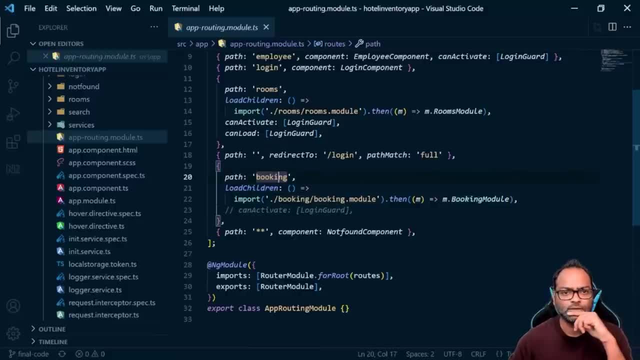 so if you see our booking is actually one of the routed component which is available here, so if you see our booking is actually one of the routed component which is available here, so i'll just change the path a little bit. so i'll just change the path a little bit. 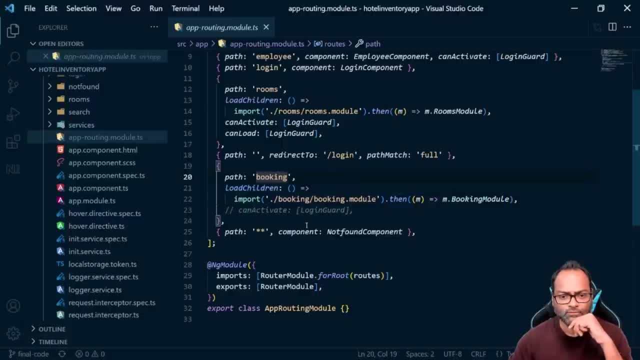 so i'll just change the path a little bit, okay, okay, okay, i'll make it as. i'll make it as i'll make it as: uh booking slash, uh booking slash, uh booking slash room, id room, id room, id. so we are booking for a specific room. 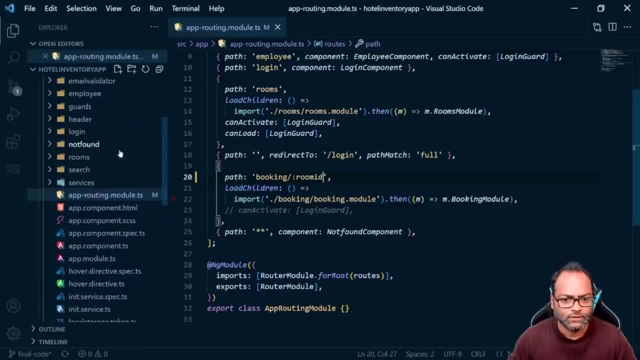 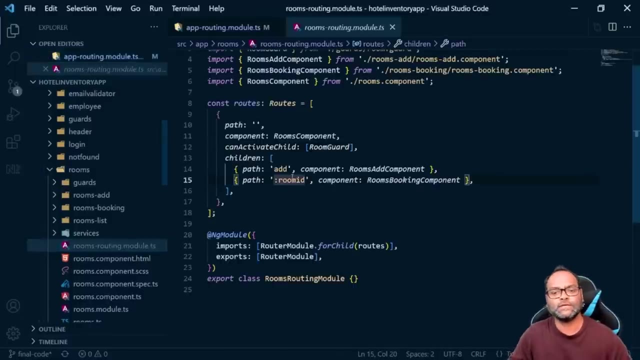 so we are booking for a specific room. so we are booking for a specific room, okay, okay, okay. and here on here on here on rooms, rooms, we had a route. so if you see, uh, we had a route. so if you see, uh, we had a route. so if you see, uh, we said okay, this should redirect to booking. 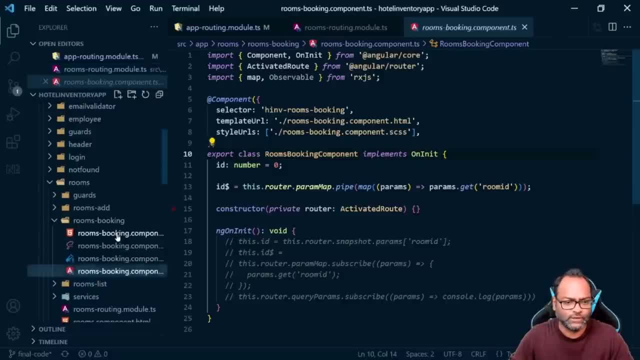 we said: okay, this should redirect to booking. we said, okay, this should redirect to booking component, component, component, and and and it's, it's another booking component, right. so it's, it's another booking component, right, so it's, it's another booking component, right? so actually, we never 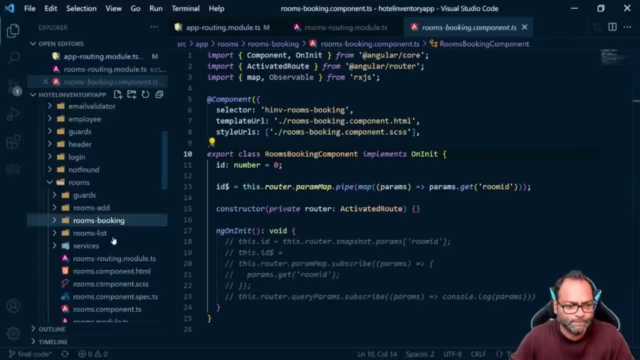 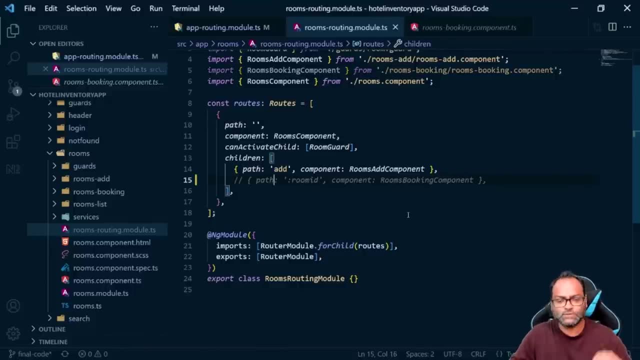 actually, we never, actually, we never, uh, did anything here. so what we'll do is: we'll remove this, we'll remove this, we'll remove this. okay, so we removed this particular route. okay, so we removed this particular route. okay, so we removed this particular route. we have booking slash. 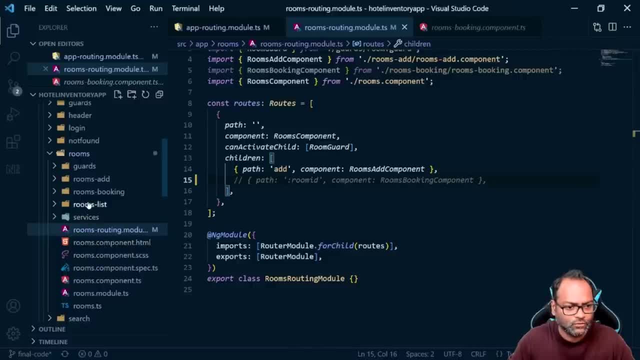 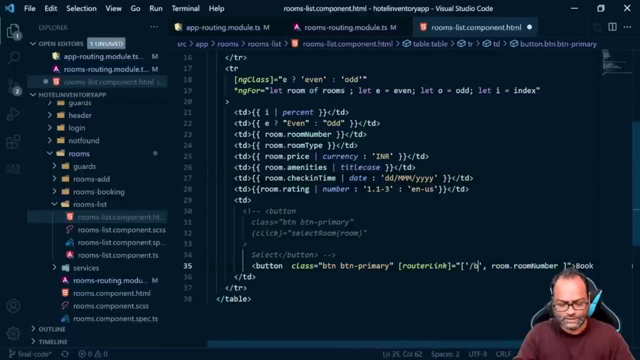 we have booking slash. we have booking slash. our room id, our room id, our room id. let's go back to the rooms list component. let's go back to the rooms list component. let's go back to the rooms list component. here and here we will say redirect to. 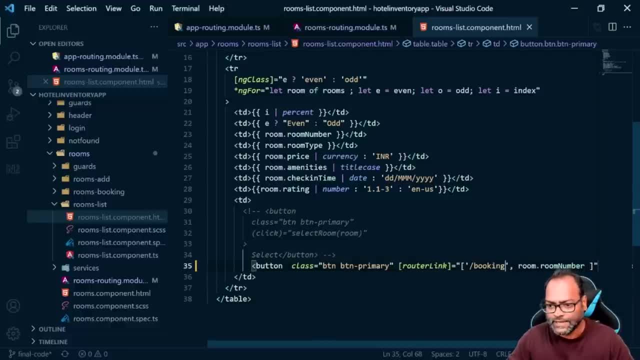 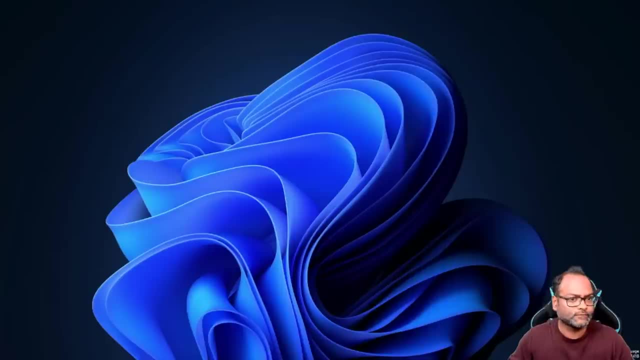 and here we will say redirect to, and here we will say redirect to: booking: slash room number. let's verify this change- slash room number. let's verify this change- slash room number. let's verify this change, and then we will proceed, and to do that we have to log in. let's. 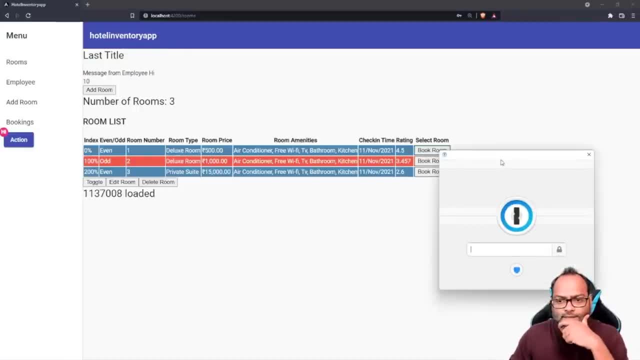 and to do that we have to log in. let's- and to do that we have to log in. let's see, see, see, and let's click on book room and let's click on book room and let's click on book room. so we are here booking slash one, right. 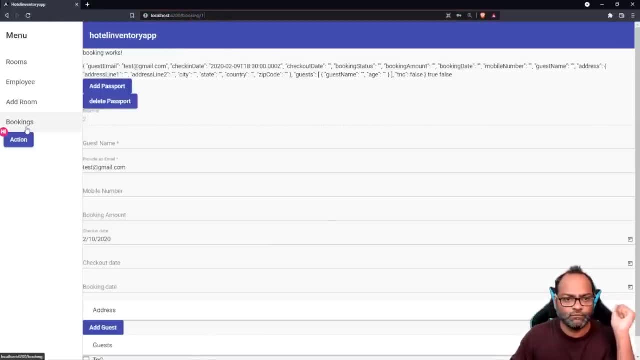 so we are here booking slash one, right? so we are here booking slash one, right? so we are getting the book. so we are getting the book, so we are getting the book. uh, a room id for which we want to book. uh, a room id for which we want to book. 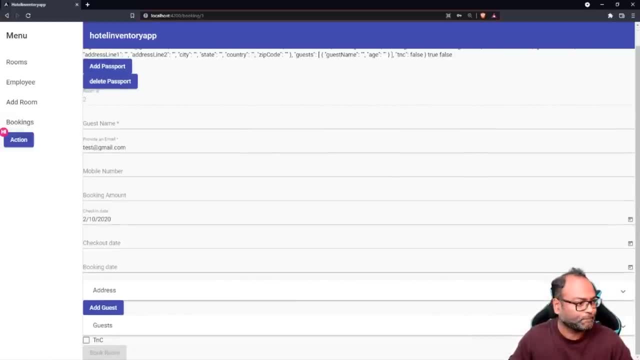 uh, a room id for which we want to book. so this is first step. we are here. so this is first step. we are here. so this is first step, we are here. next step: we will try to get this id. next step: we will try to get this id. 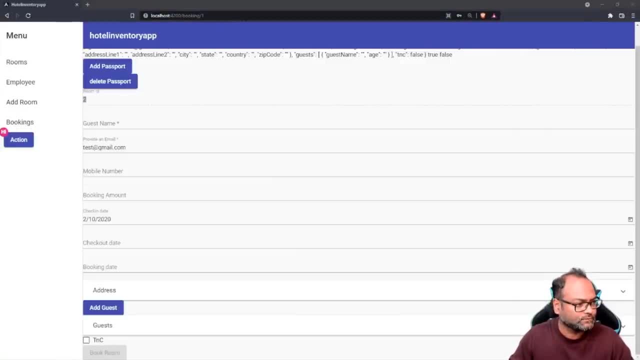 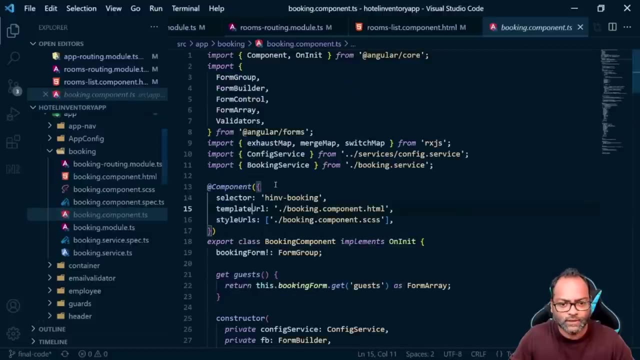 next step, we will try to get this id here with this room id. let's go back to our. let's go back to our. let's go back to our booking. booking booking: ds, ds, ds. and how we can get that data, so by using. and how we can get that data, so by using. 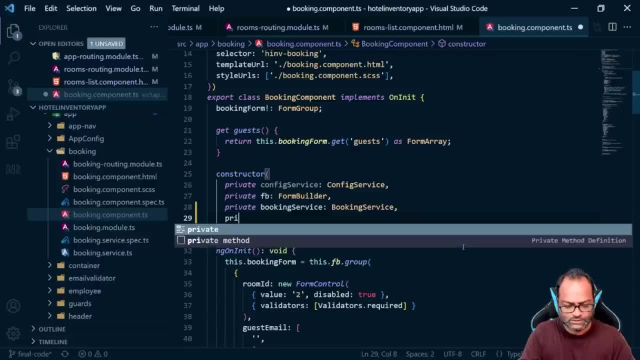 and how we can get that data. so, by using activated route. we have seen that activated route, we have seen that activated route, we have seen that we'll say: this is private and this is route and this is route and this is route. activated route, activated route, activated route, and we can, uh, do something like this: 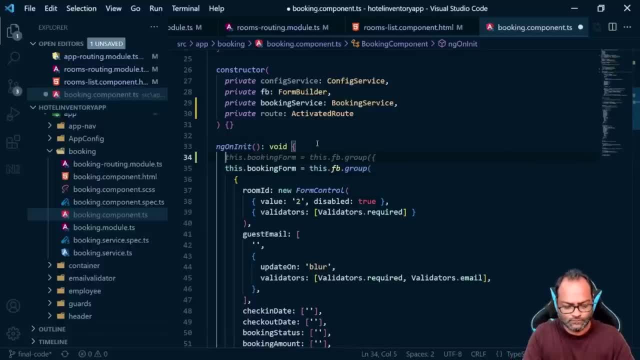 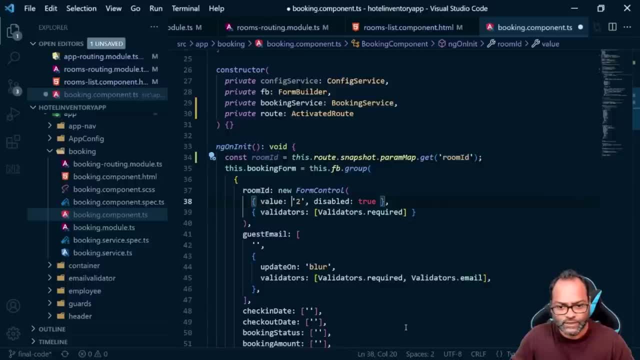 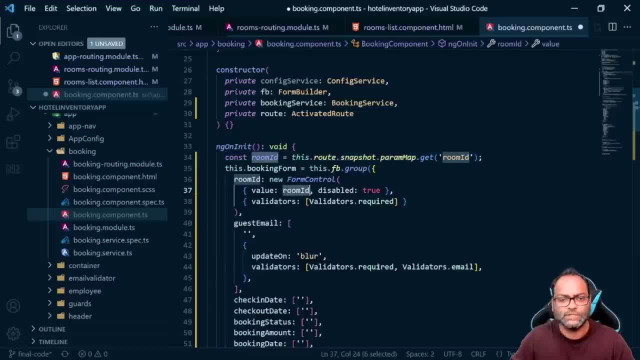 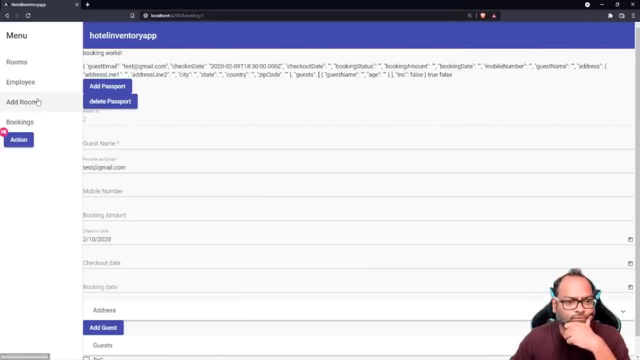 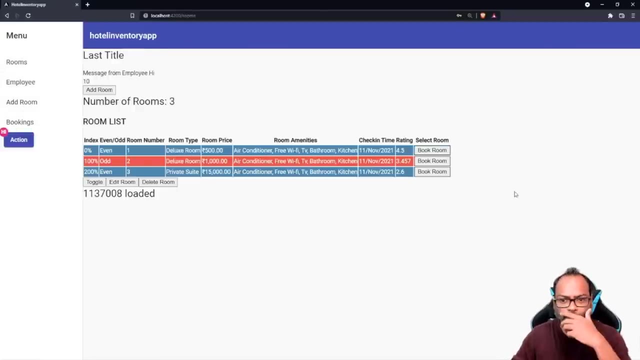 as we are inside the ngon unit. we don't as we are inside the ngon unit. we don't as we are inside the ngon unit. we don't need to do this dot room id, need to do this dot room id. need to do this dot room id. let's verify this in this behavior. 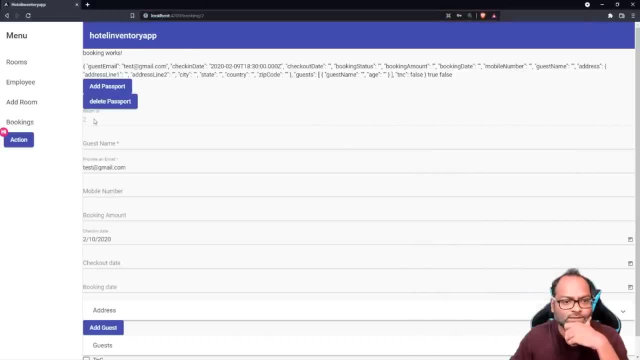 click on this, click on this, click on this, and we have this two and this two, but, and we have this two and this two but, and we have this two and this two, but you might be wondering, okay, you might be wondering. okay, you might be wondering. okay, that was the default one. let's try to. 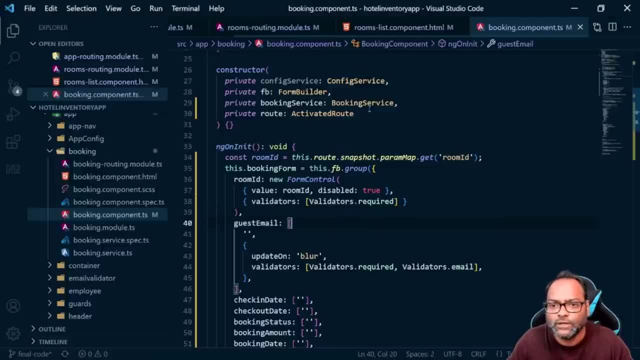 that was the default one. let's try to. that was the default one. let's try to use it for three. okay, it's still two. use it for three. okay, it's still two. use it for three. okay, it's still two. let's see what is wrong here. 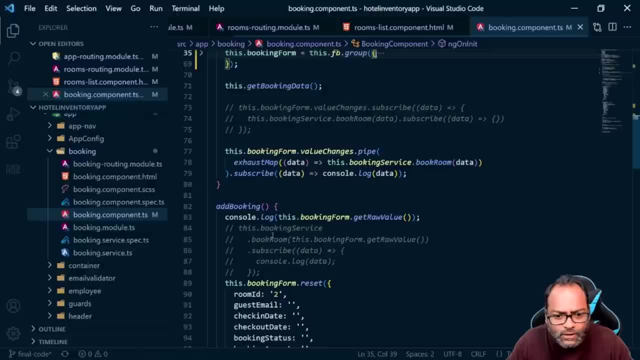 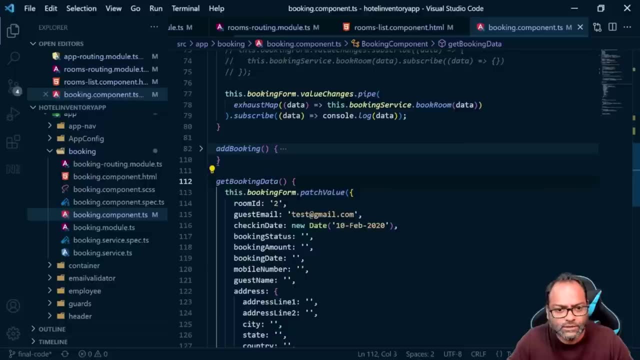 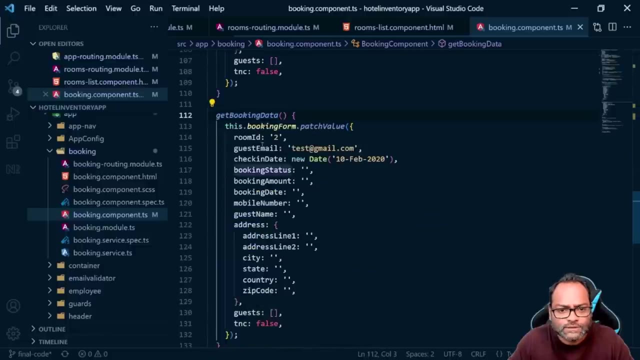 let's see what is wrong here. let's see what is wrong here. room id: this is reset. i think uh get booking data. this is reset. i think uh get booking data. this is reset. i think uh get booking data. yeah, yeah, yeah, remember, we hardcoded this. get booking data. where is this function? 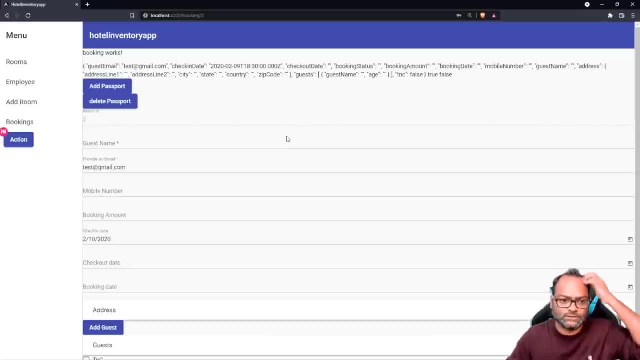 get booking data. where is this function? get booking data? where is this function? yeah, i'll remove this because we don't. yeah, i'll remove this because we don't. yeah, i'll remove this because we don't want this default value for room id. want this default value for room id. 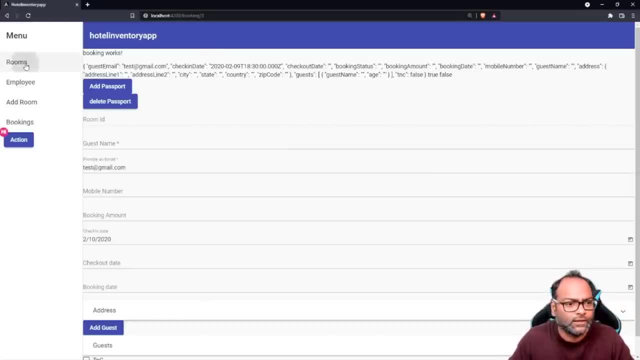 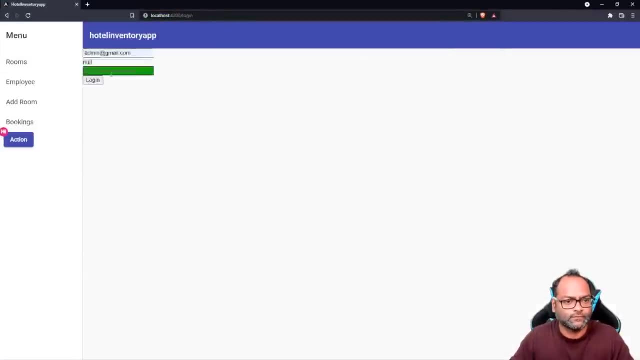 want this default value for room id. okay, okay, okay, so it's empty room id and let's go back. so it's empty room id and let's go back. so it's empty room id and let's go back to rooms, to rooms, to rooms. let's log in again. 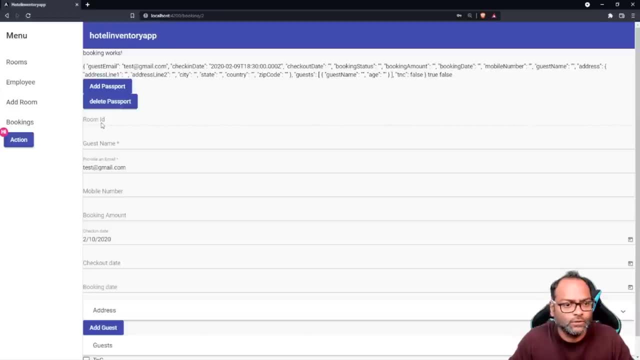 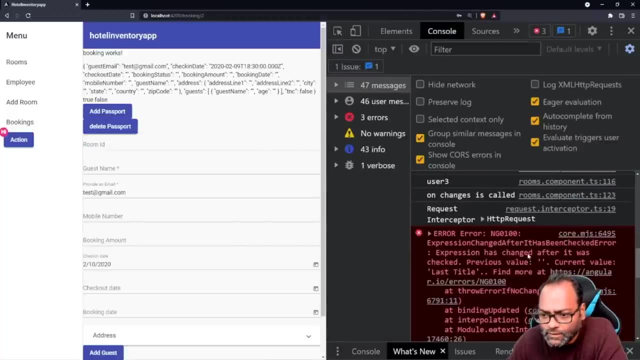 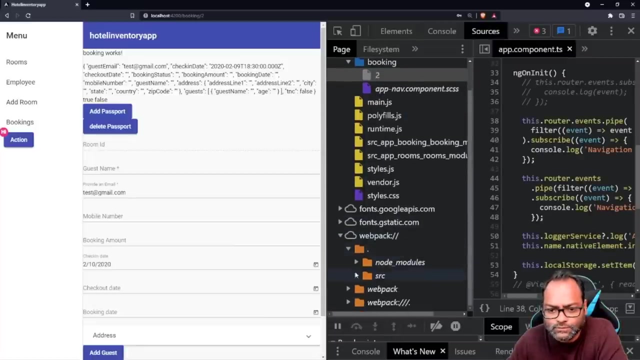 let's click on. let's click on. let's click on: room room, room. okay, somehow this value is not available. okay, somehow this value is not available. okay, somehow this value is not available. let's see why. so we can debug, we can debug, we can debug. let's go to src app. 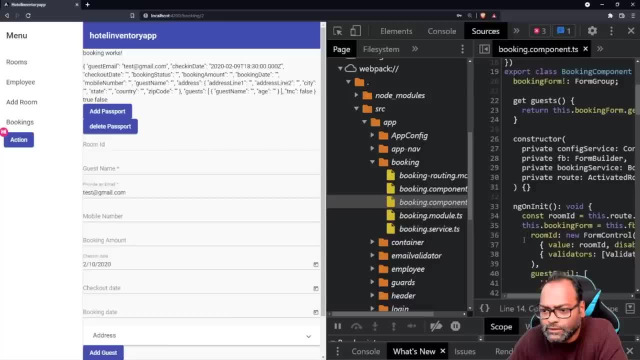 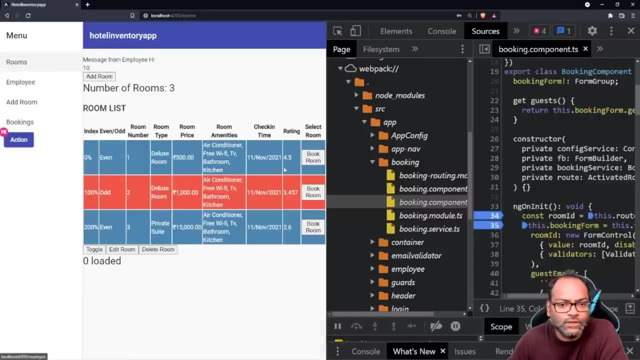 let's go to src app. let's go to src app. okay, and booking component. okay, and booking component. okay, and booking component, and this is the line number and this is the line number and this is the line number. so, let's, so, let's, so. let's see what's wrong here. 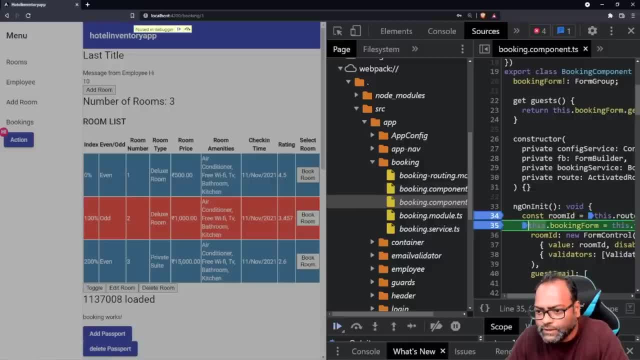 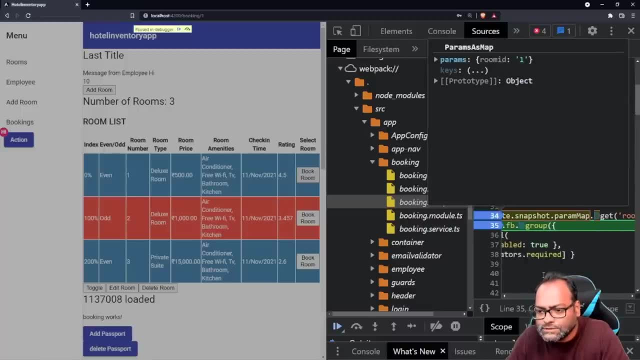 see what's wrong here. see what's wrong here: click, click, click and f10 room id is and f10 room id is and f10 room id is null. okay, param id: it says it's room id available. param id: it says it's room id available. 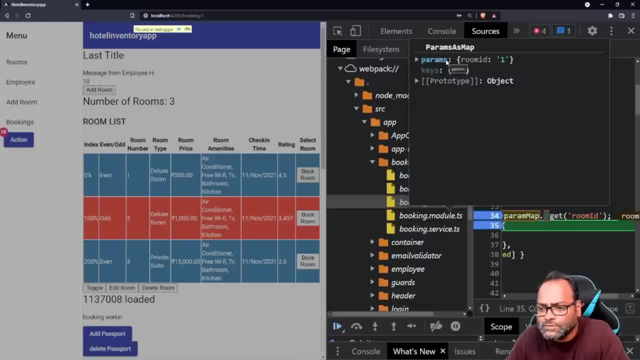 param id. it says it's room id available, but but but, params dot get room, okay, i capital okay. params dot get room, okay, i capital okay. params dot get room. okay, i capital okay. so the code was correct, the only problem. so the code was correct, the only problem. 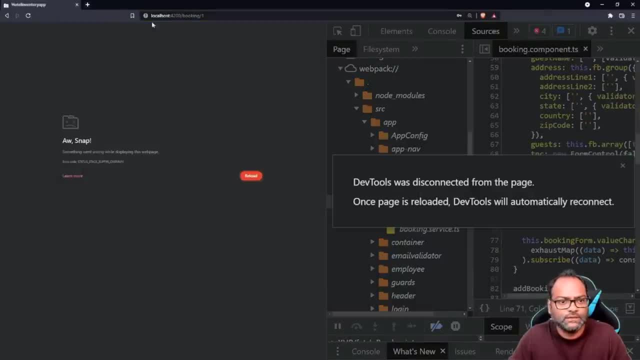 so the code was correct. the only problem is is is the uppercase and lowercase. so let's fix the uppercase and lowercase. so let's fix the uppercase and lowercase. so let's fix that, that, that, and we will say, okay, this is room. and we will say, okay, this is room. 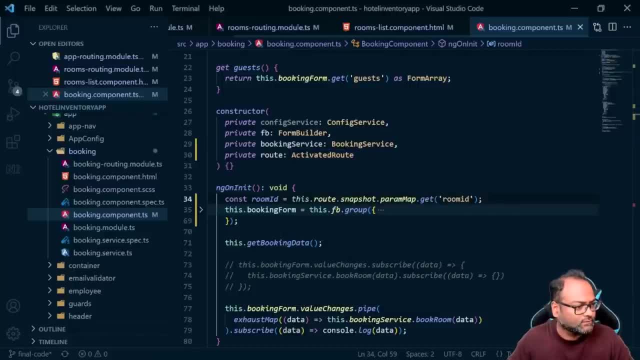 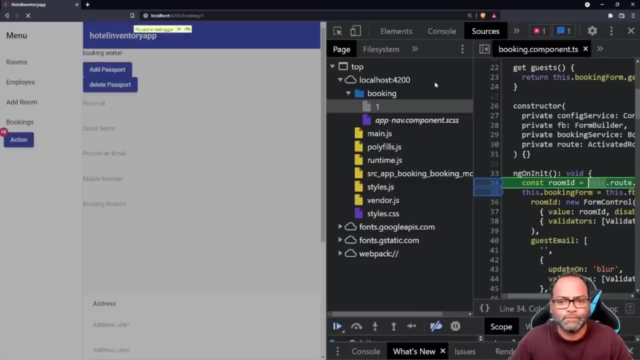 and we will say: okay, this is room, remember, the key should match. let's refresh this page now. let's refresh this page now. let's refresh this page now. and let's see, and now we have the id. and let's see, and now we have the id. 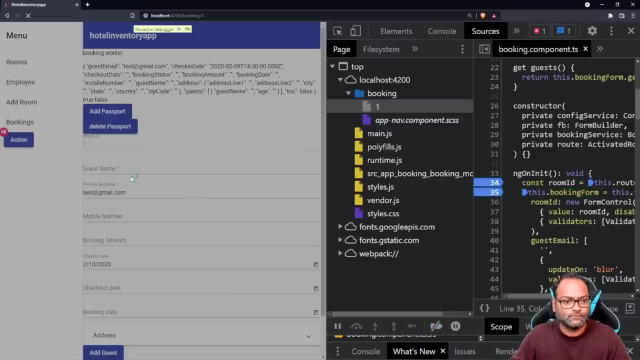 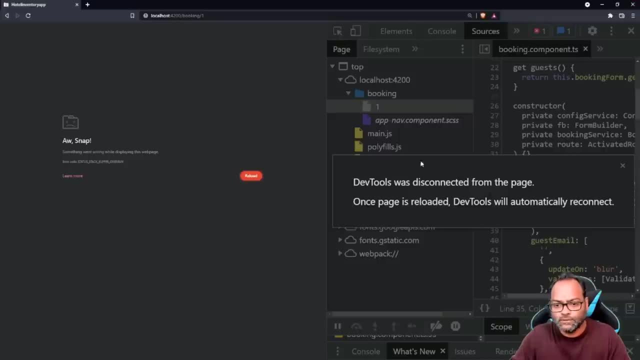 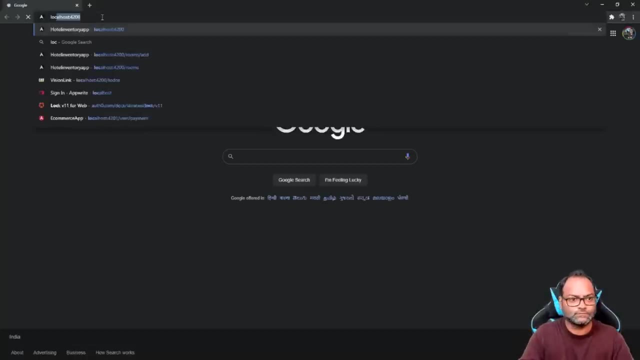 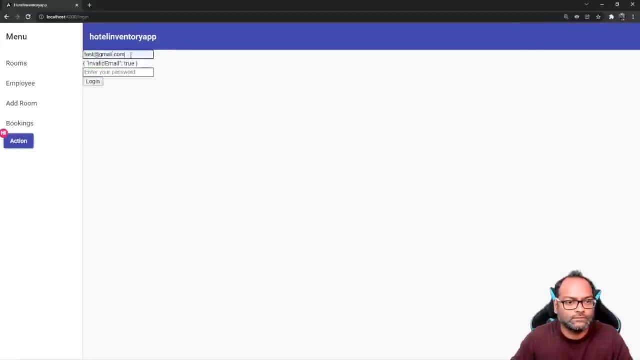 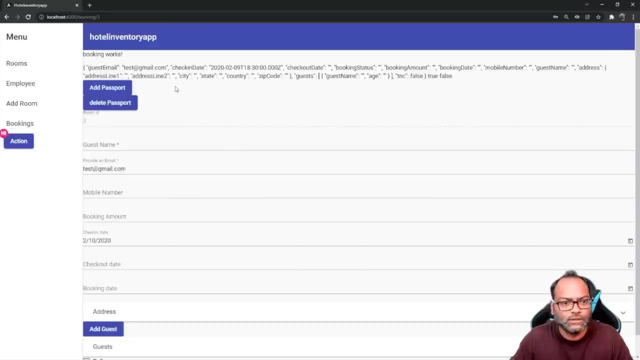 and let's see, and now we have the id, okay, great, let's move. okay, i will probably close this and okay, i will probably close this and okay, i will probably close this and open it again, open it again, open it again, and let's click on this. 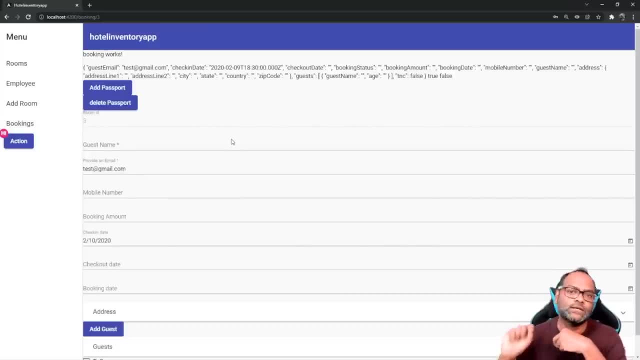 and let's click on this. and let's click on this. and works right. so we have room id3 and and works right. so we have room id3 and and works right. so we have room id3. and now we are now we are now we are booking for a specific room, so this is. 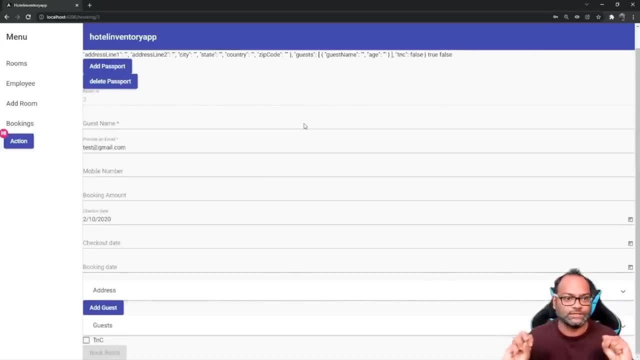 booking for a specific room. so this is booking for a specific room. so this is the second step. so first we fix it out, the second step. so first we fix it out, the second step. so first we fix it out. second, we are sick. we are saying okay, 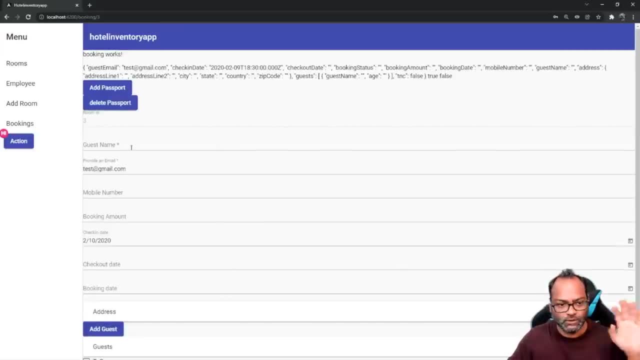 second, we are sick, we are saying okay. second, we are sick, we are saying, okay, we are. we wanted to book it for specific we are. we wanted to book it for specific we are. we wanted to book it for specific room. we are here. and now we want to add: 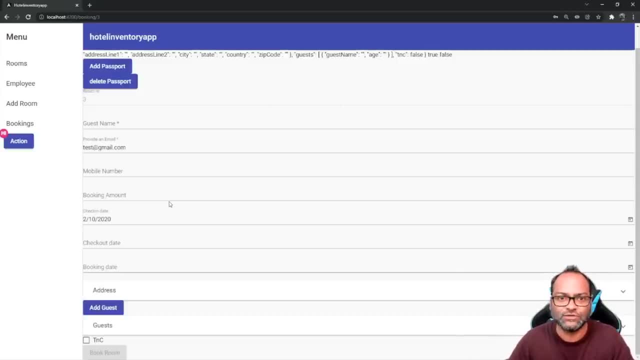 room. we are here and now we want to add room. we are here and now we want to add the guard to make sure that, in case the guard, to make sure that, in case the guard, to make sure that, in case there are some unsaved changes on this. 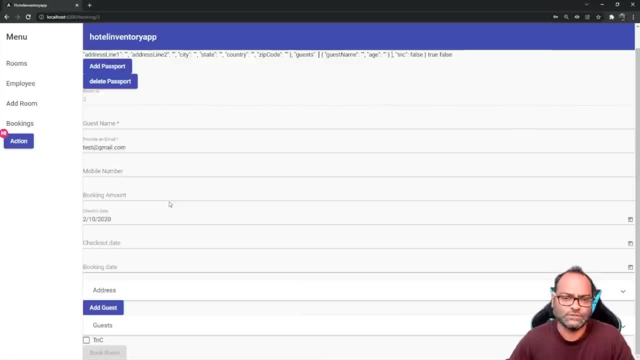 there are some unsaved changes on this. there are some unsaved changes on this form, form, form. we should send a message. we should show. we should send a message. we should show. we should send a message. we should show a message to the user that okay. a message to the user that okay. 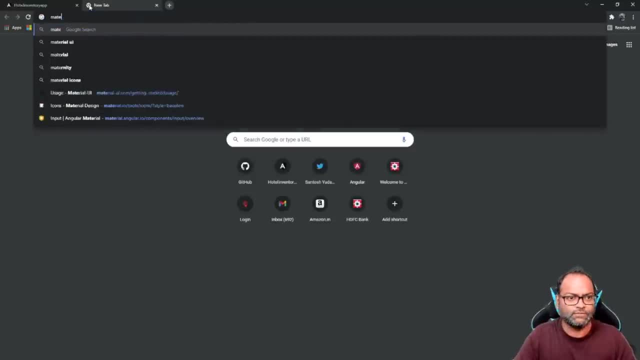 a message to the user that, okay, there are some unsaved changes. so let's, there are some unsaved changes. so let's, there are some unsaved changes. so let's see if we can use some material control, see if we can use some material control, see if we can use some material control to do that. so i think material has. 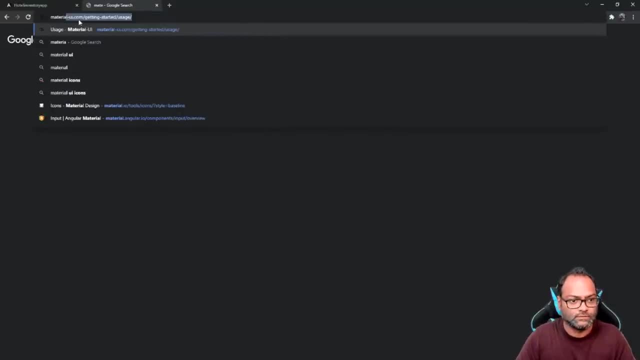 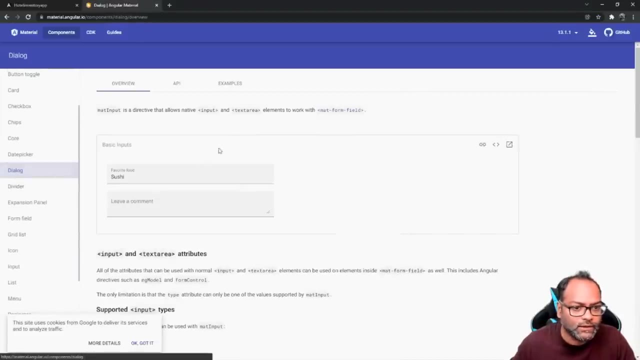 to do that. so i think material has to do that. so i think material has something for us material, something for us material, something for us material- angular material, angular material, angular material. so we can use this, so we can use this, so we can use this. let's see. 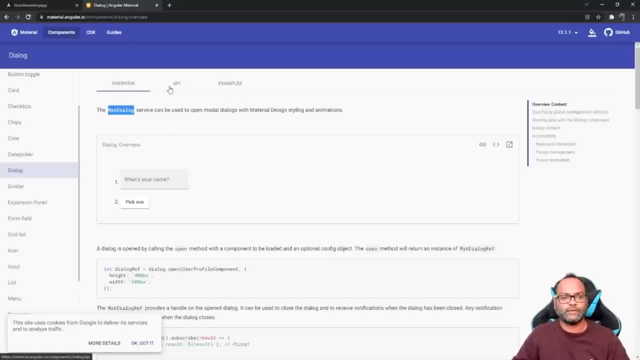 let's see. let's see, yeah, we can use this matte dialogue to: yeah, we can use this matte dialogue to: yeah, we can use this matte dialogue to show and dialogue, saying you have some show and dialogue. saying you have some show and dialogue saying you have some unsaved changes. 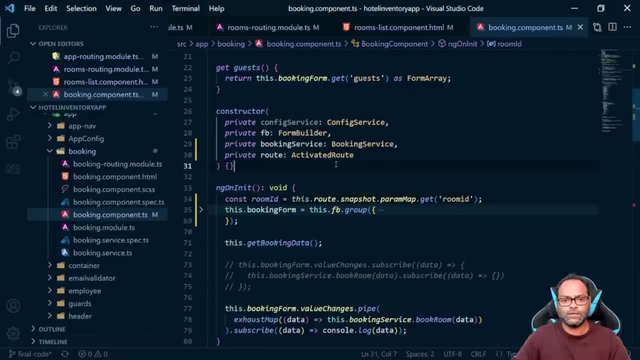 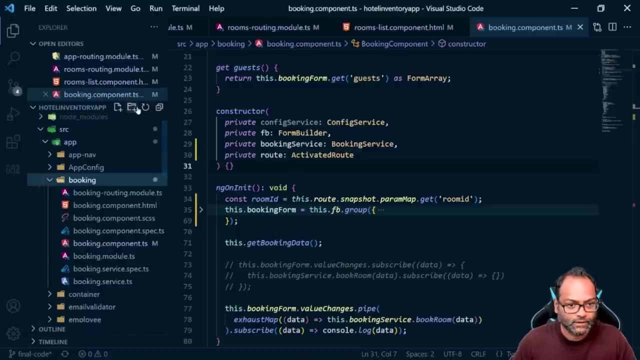 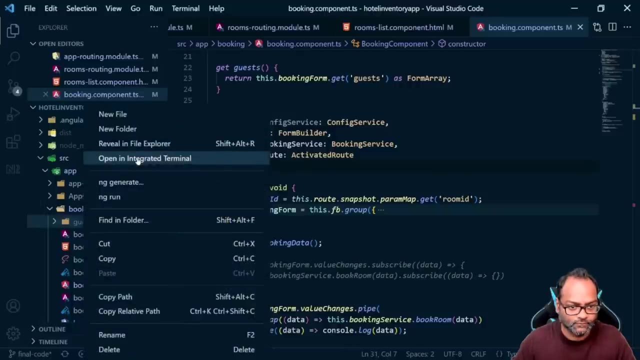 unsaved changes. unsaved changes. but let's do it later. first let's add: but let's do it later, first let's add, but let's do it later, first let's add: uh uh, uh card. here we will create, here we will create, here we will create. 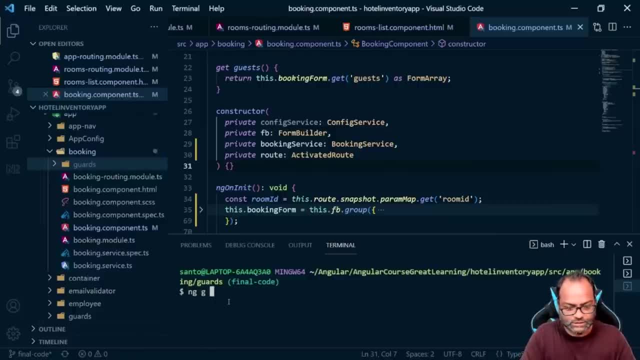 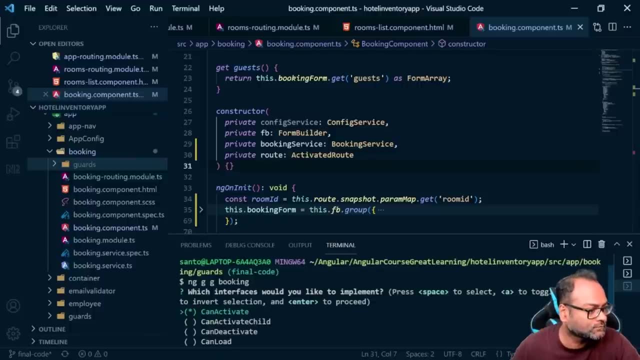 a guard and i'll say this is ng a guard. and i'll say this is ng a guard and i'll say this is ng g, g and this is booking guard. and what we need is: we just need can, and what we need is: we just need can. 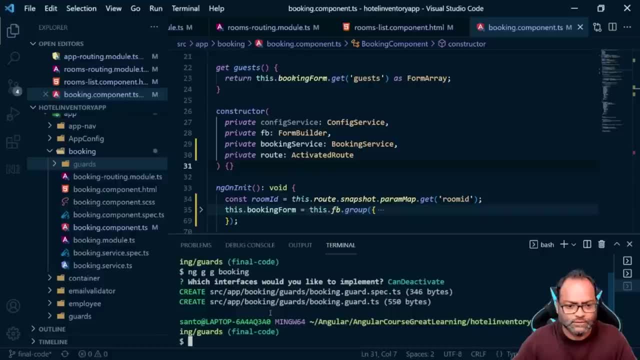 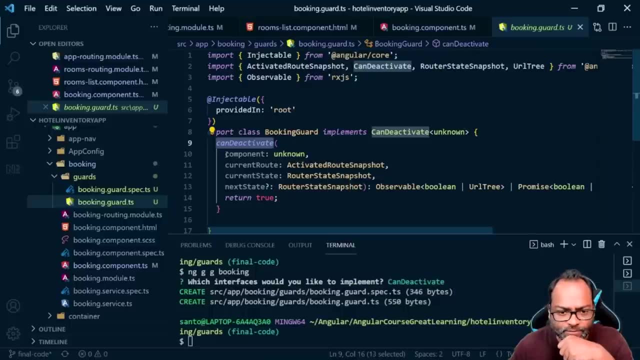 and what we need is we just need can reactivate and that's it reactivate, and that's it reactivate, and that's it. so you can see in can deactivate. we are so you can see. in can deactivate, we are so you can see. in can deactivate. we are getting one extra parameter. 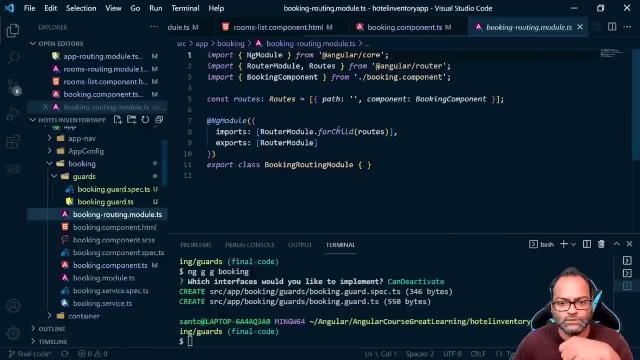 getting one extra parameter. getting one extra parameter. so we have something known as component. so we have something known as component, so we have something known as component. so this is the routed component. so we so this is the routed component. so we so this is the routed component, so we will pass this booking component. 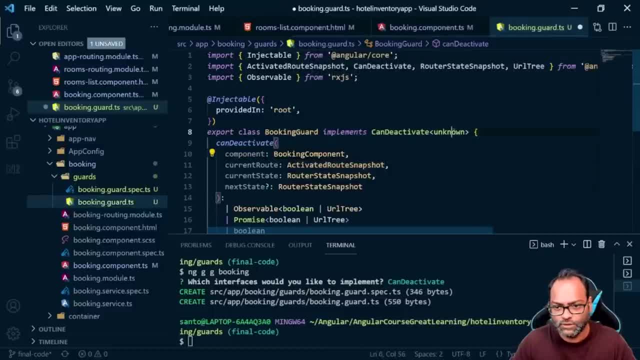 will pass this booking component. will pass this booking component as one of the parameter here, which is as one of the parameter here, which is as one of the parameter here which is unknown, unknown, unknown, and same here, so let's go ahead. and and same here, so let's go ahead and 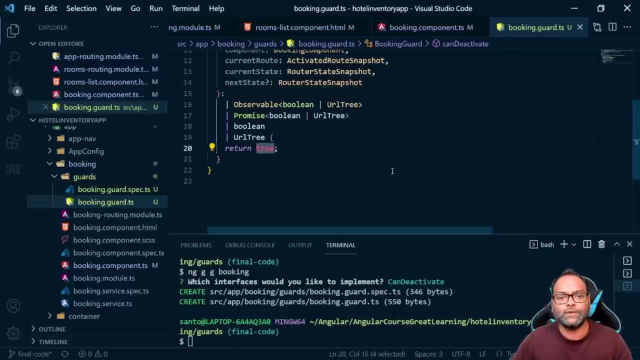 and same here. so let's go ahead and see what we can achieve using this, see what we can achieve using this, see what we can achieve using this. so now, uh, we can. so now, uh, we can. so now, uh, we can put and check, put and check. 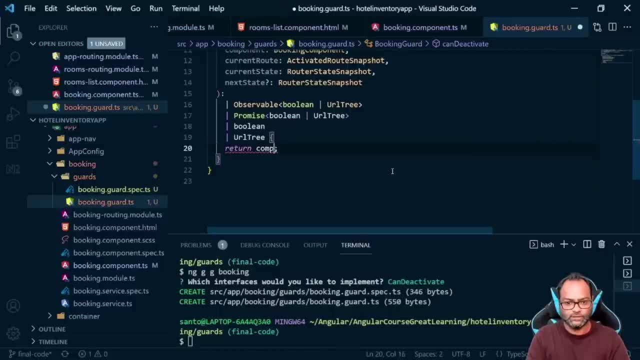 put and check so i can say uh in case this. so i can say uh in case this, so i can say uh in case this. component dot the property which is component dot the property which is component dot the property which is booking form, booking form, booking form, dot uh if it is dirty. 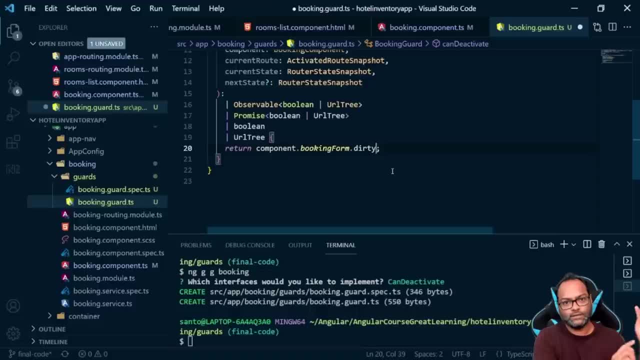 dot uh if it is dirty. dot uh if it is dirty. so. so. so, if it is dirty, so go ahead and so yeah, so it's. if it is dirty we should, so yeah, so it's. if it is dirty we should, so yeah, so it's. if it is dirty. we should not allow the user to exit. 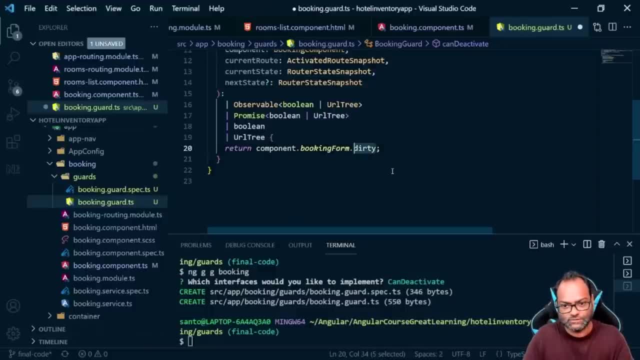 not allow the user to exit. not allow the user to exit. if it is pristine, we should allow you. if it is pristine, we should allow you. if it is pristine, we should allow you. user to exit. so i'll just go ahead. and user to exit, so i'll just go ahead and 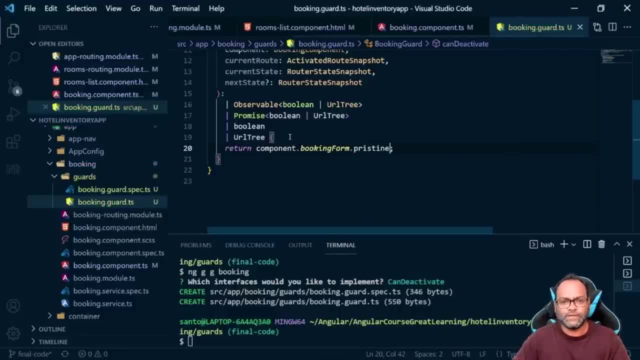 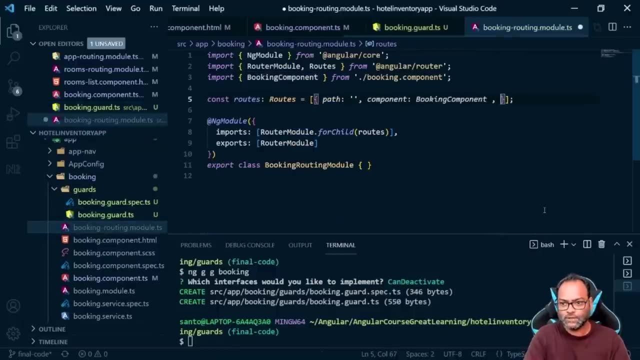 user to exit. so i'll just go ahead and say: pristine, and let's verify by applying this card, and let's verify by applying this card, and let's verify by applying this card, so we will, so we will, so we will apply this. can this, can? this can deactivate. 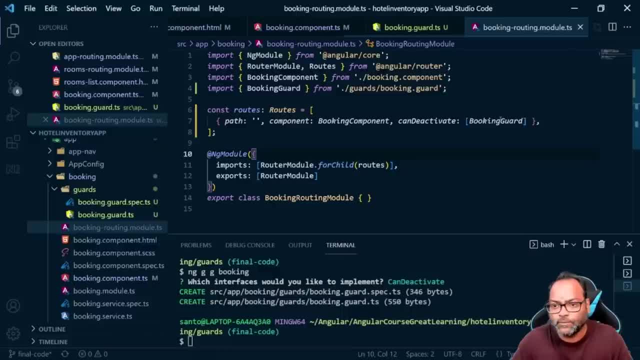 deactivate. deactivate to this booking guard. so to this booking guard, so to this booking guard. so this and pass the booking again. it's an this. and pass the booking again. it's an this and pass the booking again. it's an error. so you can pass multiple error. so you can pass multiple. 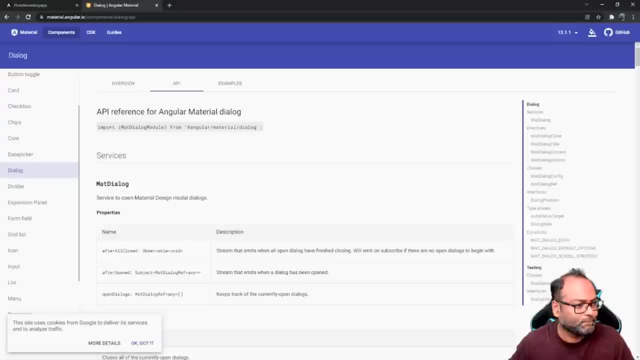 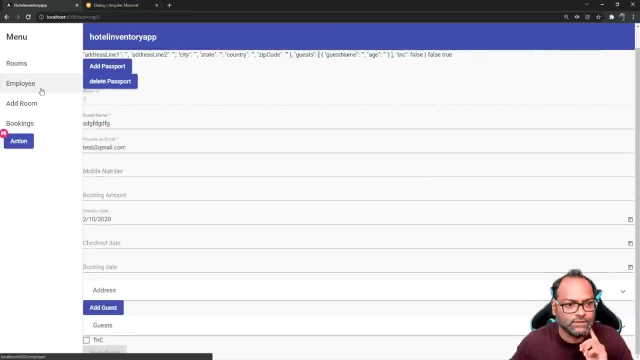 error, so you can pass multiple. let's verify this functionality so far. let's verify this functionality so far. let's verify this functionality so far, and then we'll add the dialog, and then we'll add the dialog, and then we'll add the dialog. so, uh, we have this. let's try to click. 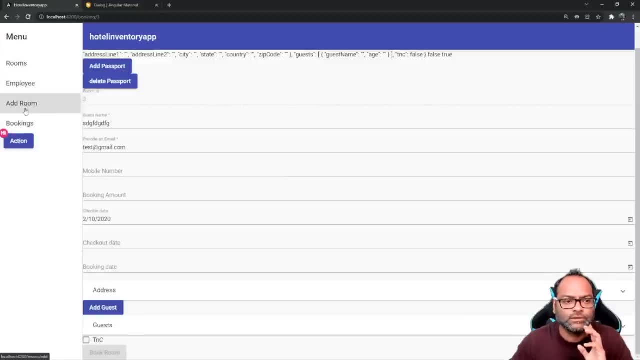 so, uh, we have this, let's try to click. so, uh, we have this, let's try to click somewhere else, somewhere else, somewhere else. we are not able to redirect. we are not able to redirect. we are not able to redirect, right, so you can see, i cannot um. 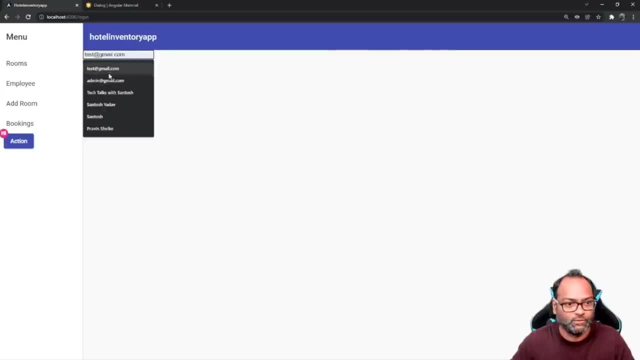 right, so you can see i cannot. um, right, so you can see i cannot. um, let's, let's, let's. again with login, you might be wondering again with login. you might be wondering again with login. you might be wondering: okay, probably, uh, because the. okay, probably uh, because the 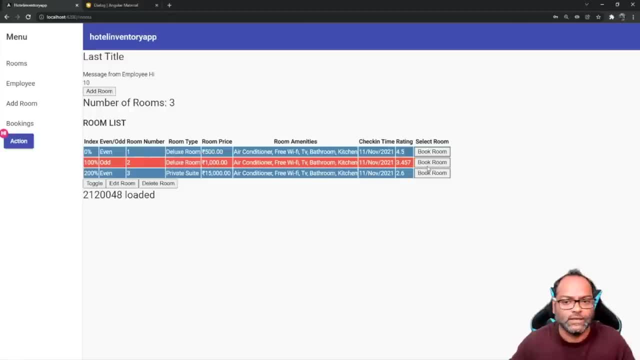 okay, probably, uh, because the state has reset. we are not able to, but state has reset. we are not able to, but state has reset. we are not able to. but let's, let's, let's log in and see log in and see log in and see right, so we have three. let's enter. 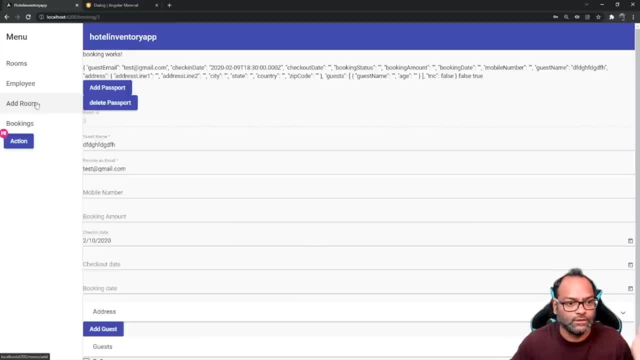 right, so we have three. let's enter right, so we have three. let's enter something. let's try to move, and we are something. let's try to move and we are something. let's try to move and we are not able to do it. not able to do it. 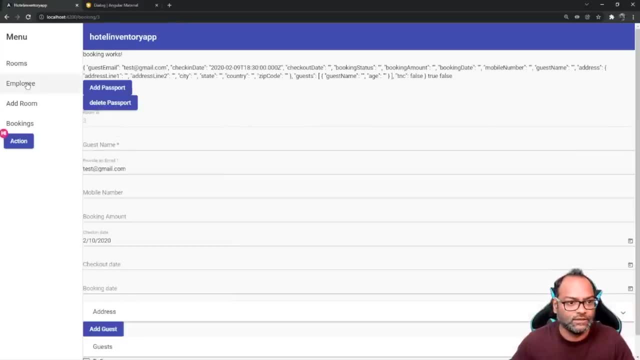 not able to do it, let's reset this form so i'll refresh. so let's reset this form, so i'll refresh. so let's reset this form, so i'll refresh. so it's in pristine state. let's try to move. it's in pristine state, let's try to move. 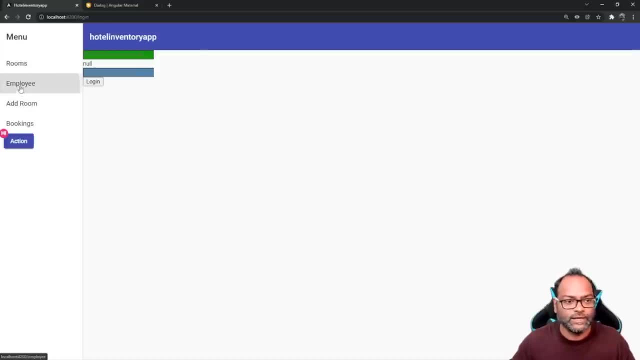 it's in pristine state. let's try to move. uh so, uh, so, uh so, let's see we are able to redirect. let's see we are able to redirect. let's see we are able to redirect. this is it, this is it, this is it so? we- it means our. 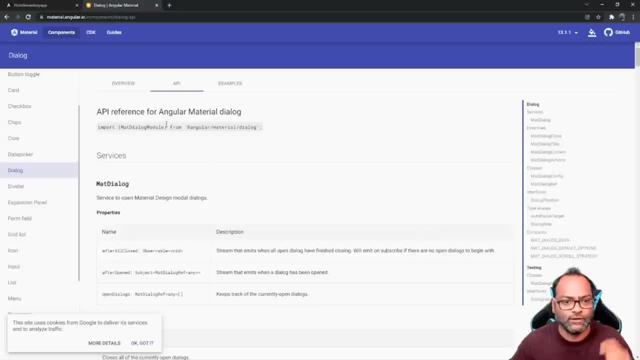 so we. it means our, so we. it means our guard is working perfectly fine. let's guard is working perfectly fine, let's guard is working perfectly fine. let's put the dialog now. put the dialog now. put the dialog now. so here let's see some example open. 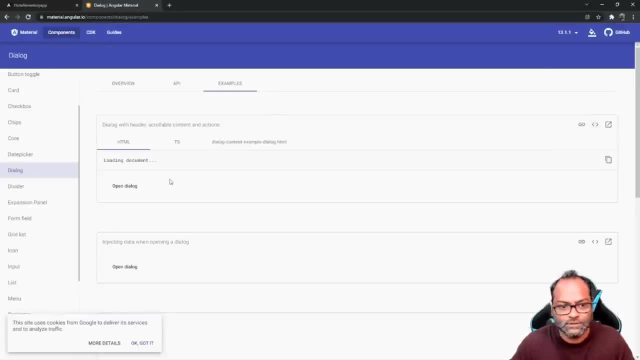 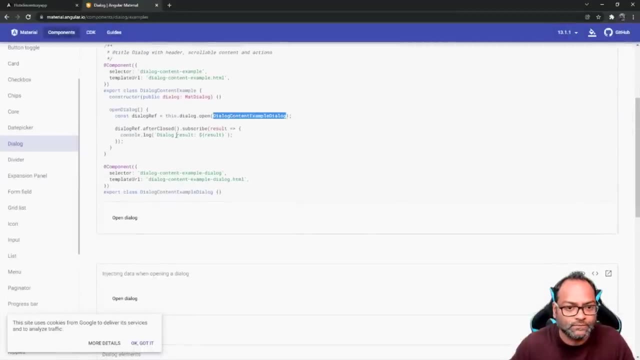 so here let's see some example open. so here let's see some example: open dialog okay, dialog, okay, dialog, okay, cancel, let's cancel, let's cancel. let's see the code, see the code, see the code. and open dialog and open dialog and open dialog. we can pass some example dialog here. 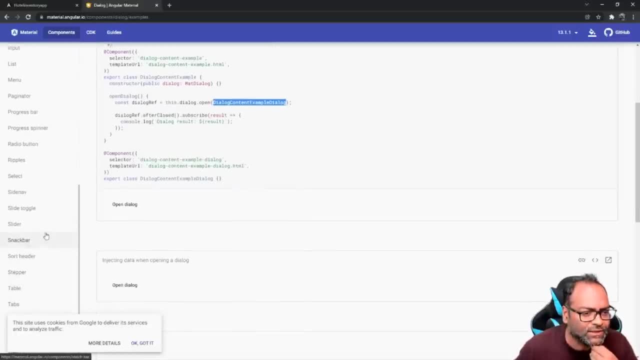 we can pass some example dialog here. we can pass some example dialog here: or let's uh, or let's uh, or let's uh, not do this. i think there is another uh, not do this. i think there is another uh, not do this. i think there is another uh- control which. 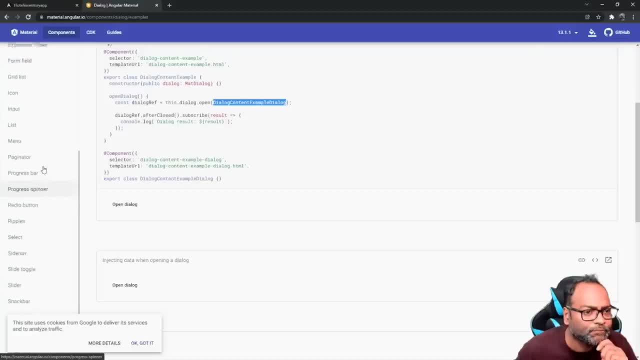 control, which, control which, where we can just directly pass the, where we can just directly pass the, where we can just directly pass the message. uh, where is that message? uh, where is that message? uh, where is that? divider date picker chips- no chip, no. divider date picker chips- no chip, no. 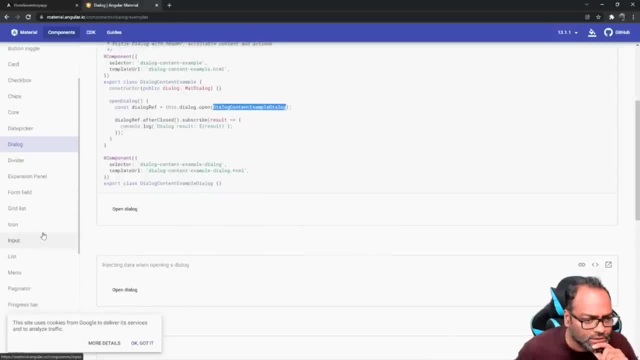 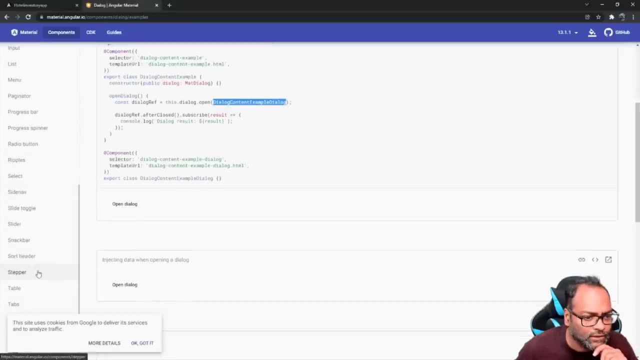 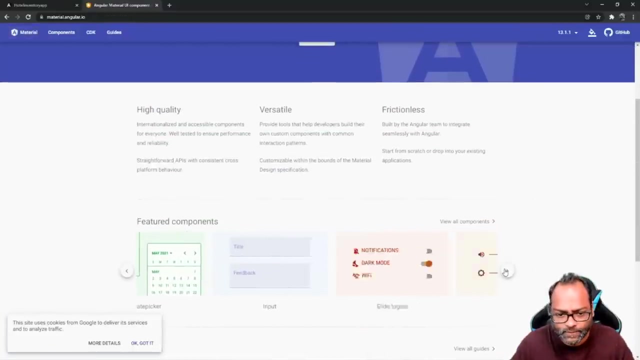 divider date: picker chips: no chip, no chips. expansion. let me just go to. let me just go to. let me just go to the default page. i think there are there, the default page. i think there are there the default page. i think there are. there should be slider buttons. 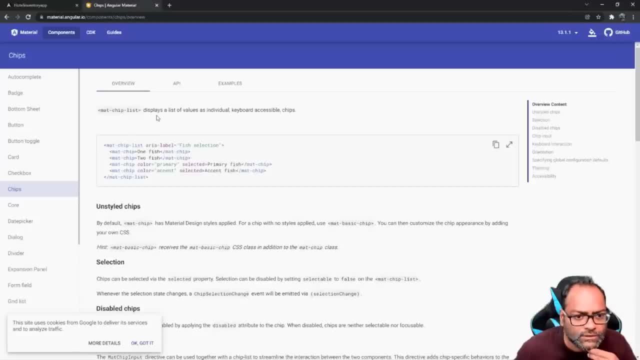 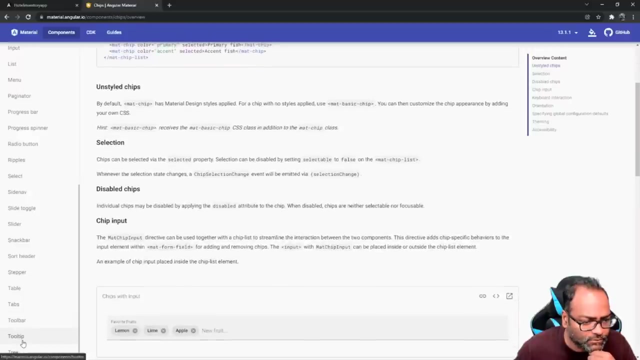 okay, okay, no, we are not looking for chips. we are no, we are not looking for chips. we are no, we are not looking for chips. we are looking, looking, looking for, for. for you know, progress bar advice: okay, okay, okay. stepper tabs- toolbar tooltip. stepper tabs- toolbar tooltip. 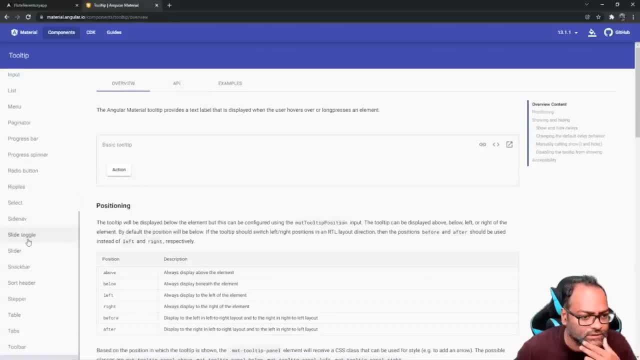 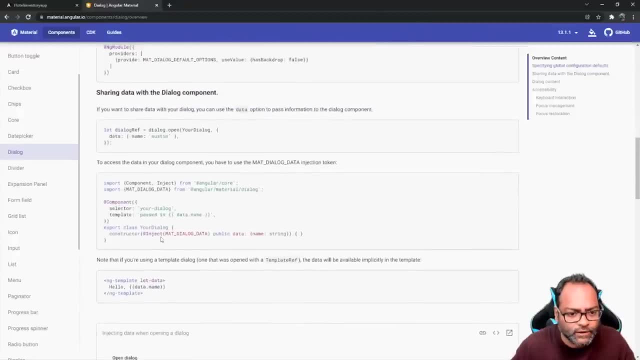 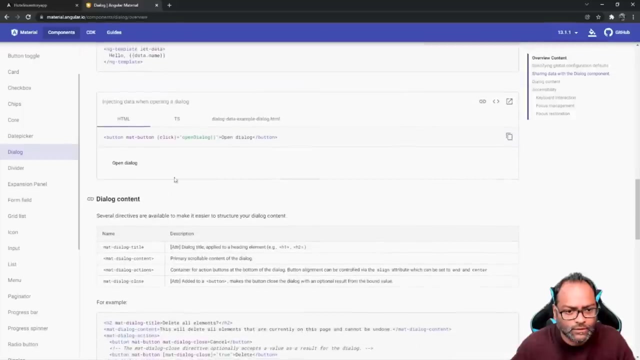 stepper tabs: toolbar tooltip tooltip. tooltip tooltip. okay, let's see, okay, let's see, okay, let's see, okay, this is not. let's see there should be a way to. let's see there should be a way to. let's see there should be a way to this. 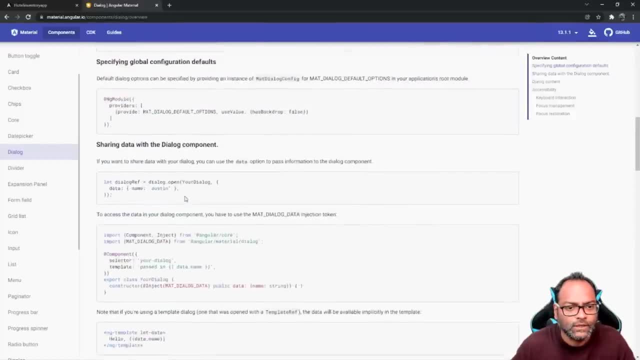 this, this and pass and pass and pass some, some, some data. okay, so we will. we will be using this data. okay, so we will. we will be using this data. okay, so we will. we will be using this one. we will be using dialog one. we will be using dialog. 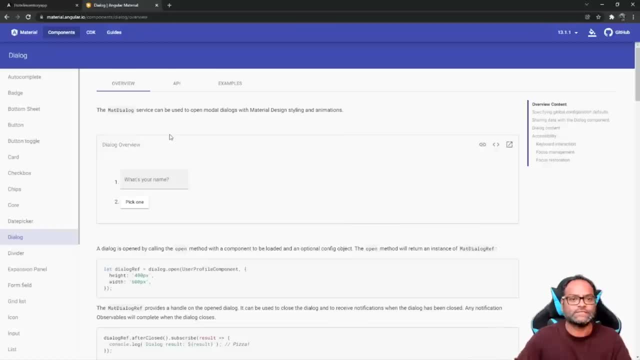 one. we will be using dialog to uh show that. okay. to uh show that. okay. to uh show that. okay, we'll show the message that, okay, you we'll show the message that, okay, you we'll show the message that, okay, you have some unsafe changes. this is what we. 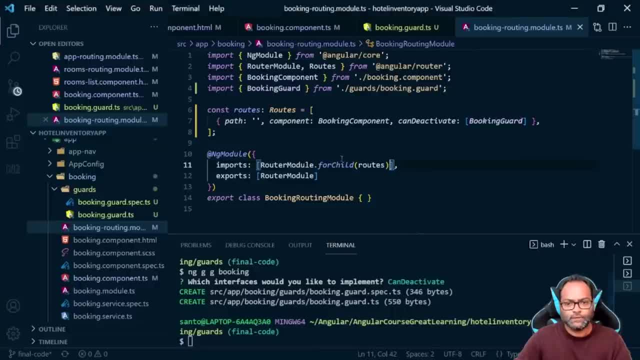 have some unsafe changes. this is what we have: some unsafe changes. this is what we are going to do here now. let's go back to the booking guard. now. let's go back to the booking guard. now. let's go back to the booking guard and here let's use. 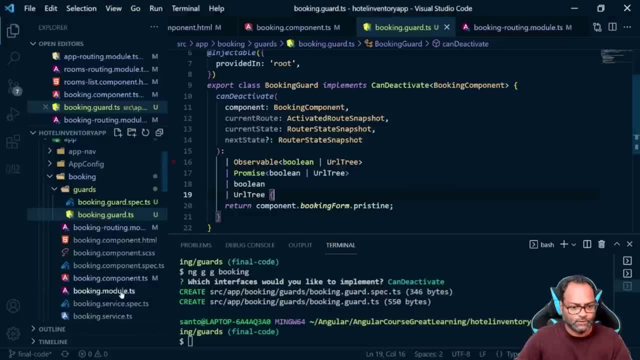 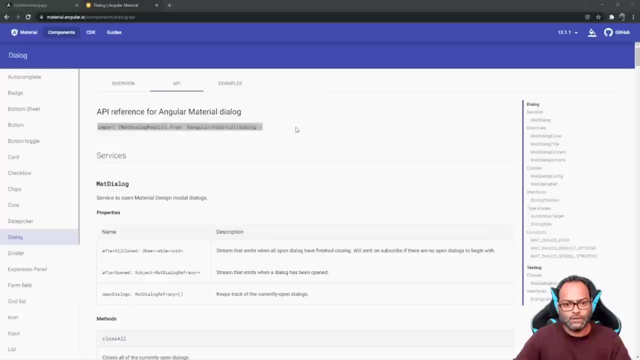 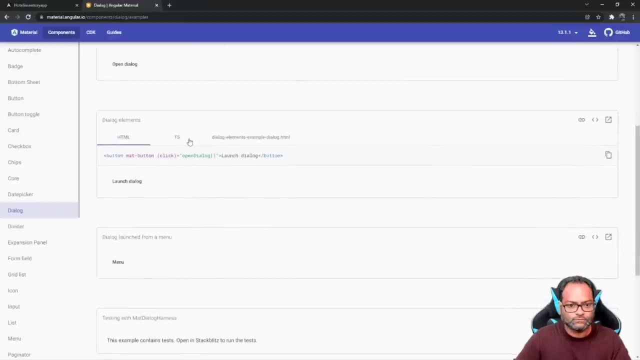 and here let's use, and here let's use import the api mat dialog module, mat dialog module, mat dialog module, and, and and let's go to the example. so it says, okay, you have to pass an. so it says okay, you have to pass an. so it says, okay, you have to pass an component. so let's create a component. 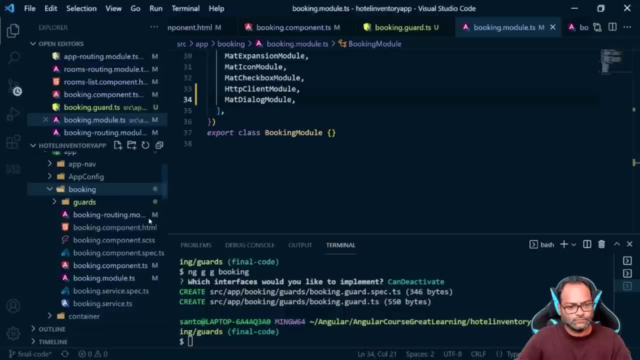 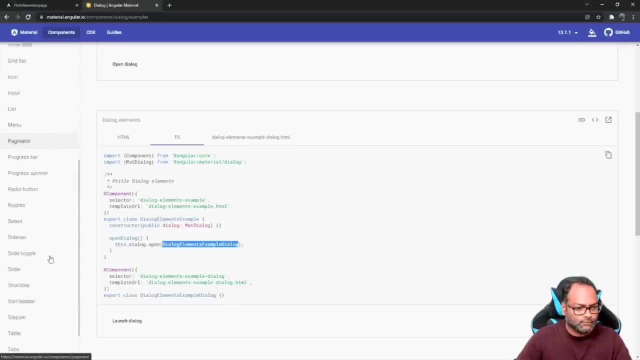 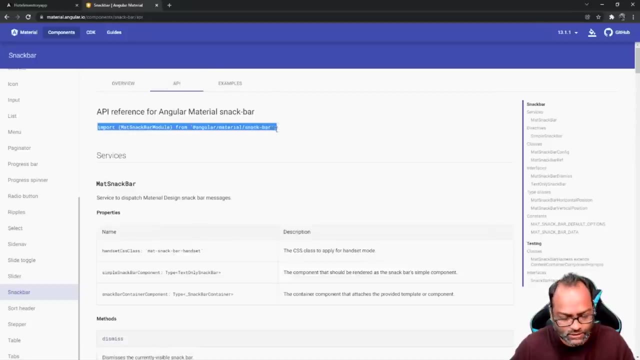 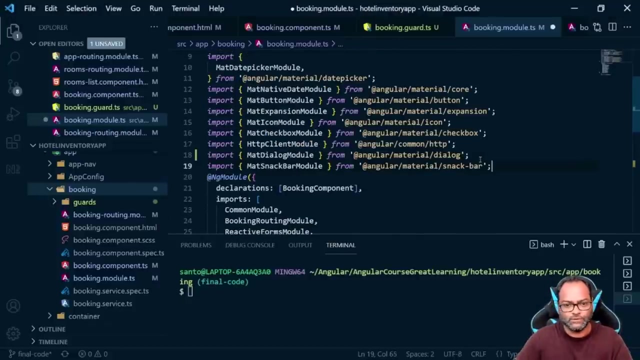 okay, okay, we can use snackbar, okay, this, this will be, uh, the easiest one. so snackbar is something where you can display a message like this. so let's say here: right, so we can display a message. it's a simple api, then dialog, because we don't need to create a component, but we will add this: uh, try to use. 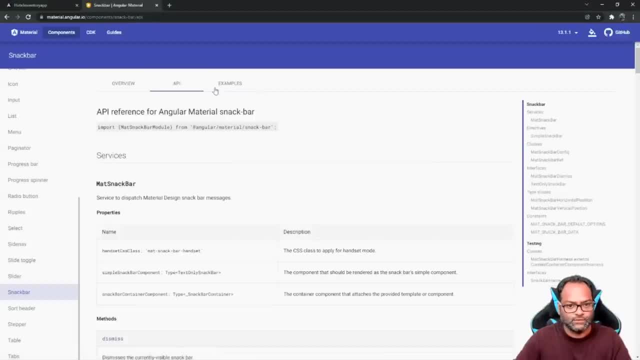 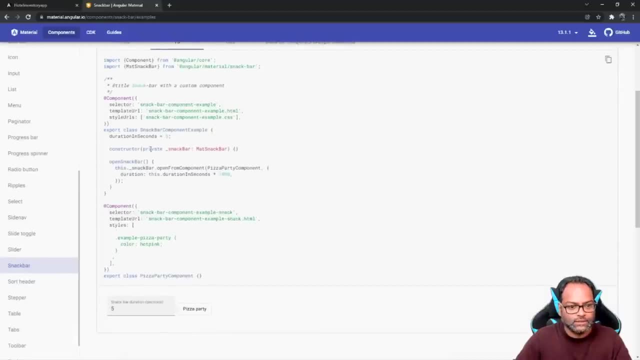 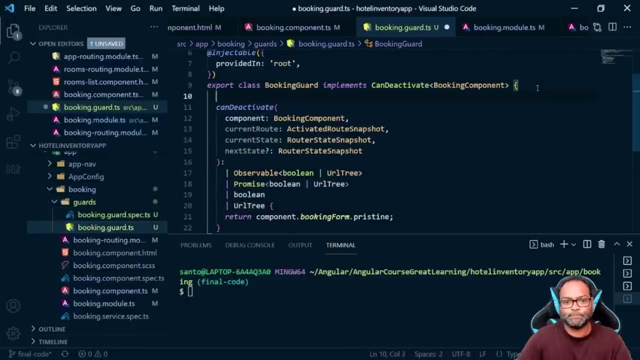 dialog module, if you can, if you want to try this out. and here, uh, in the thing is, you can just inject a snake mat, snake bar into your service. so let's do that, we'll do a constructor and then inject the snackbar. and here we can do. 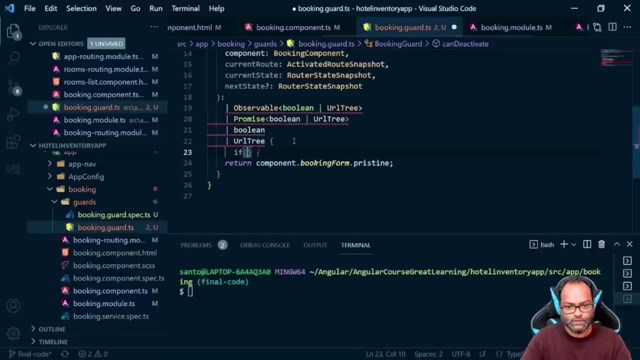 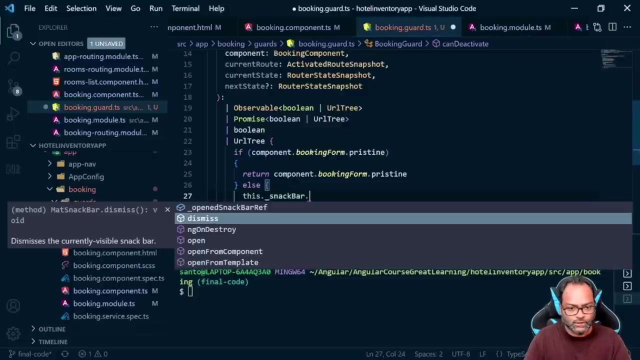 before we return this message, right? so we'll say: if uh component is pristine, return this. else what we are going to do is we are going to return false anyways, but we will open this dot. so snackbar dot. uh from template open, we can open and then we can say okay. 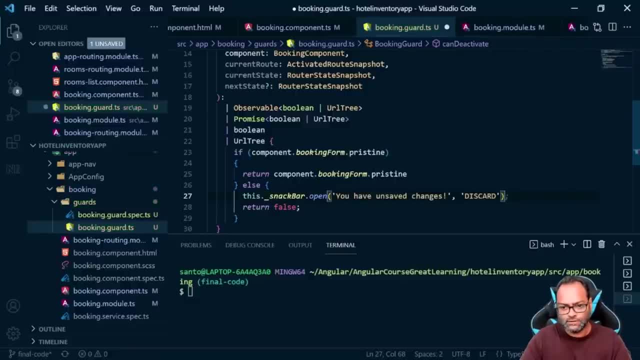 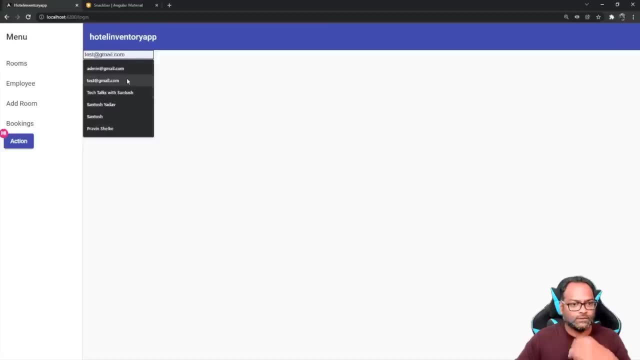 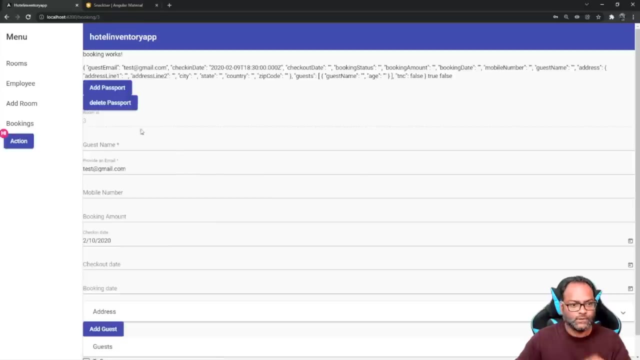 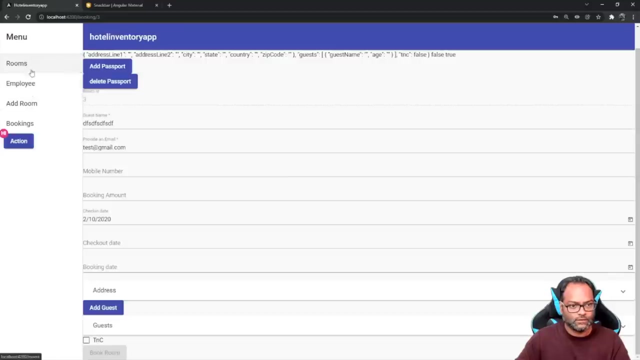 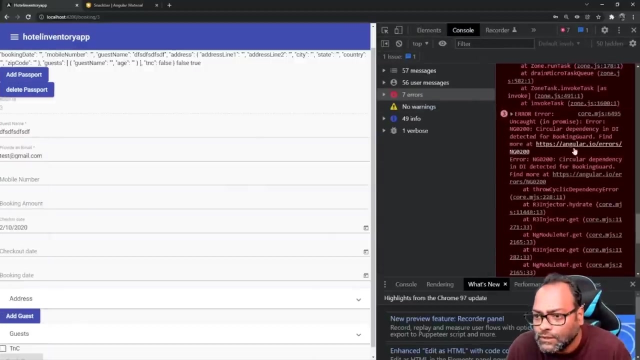 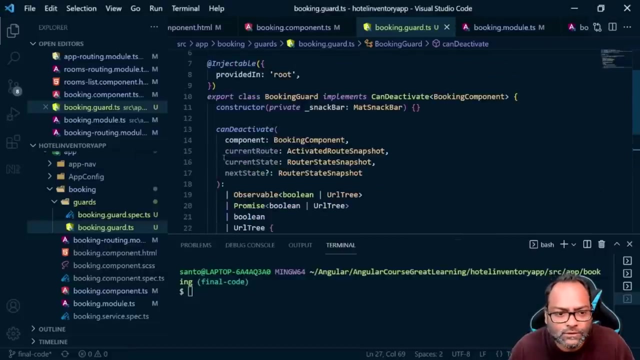 you have unsaved changes and that's it. let's verify this one click, so admin, admin, and click on booking a room, and let's do this and try to move. okay, let's see what's wrong. so, circular dependency for booking guard. okay, so how, the how is that a circular dependency? 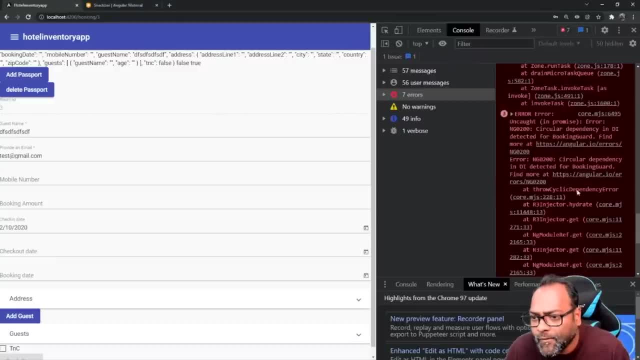 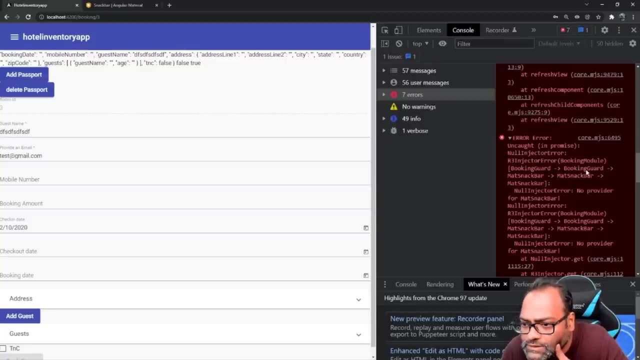 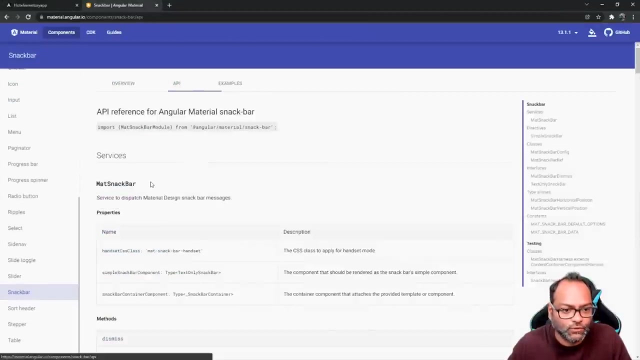 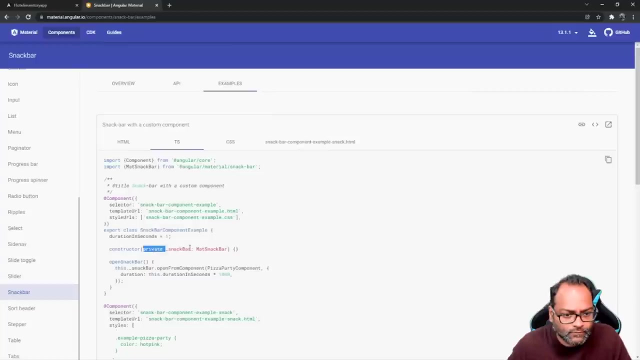 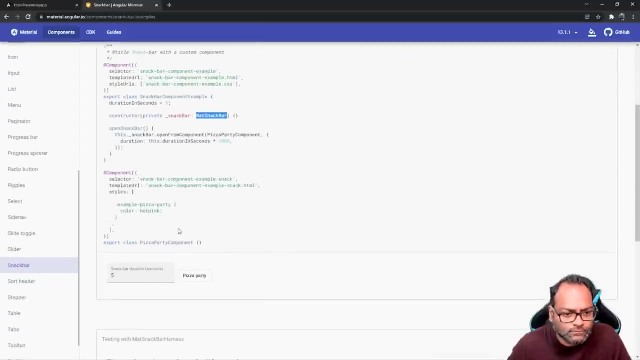 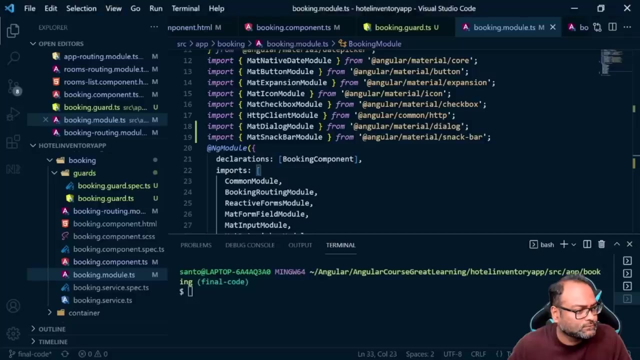 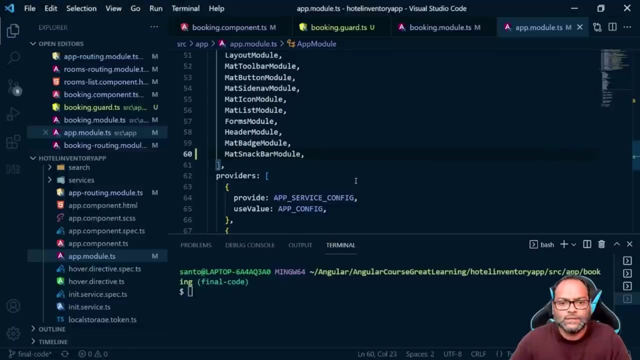 book module it says booking guard is no provider for matt's neck bar. okay, let's see. let's see the api. so in case we want to, we have to provide something. so kubectl. so we have to actually just add mat snack snagbar module into app module as well, somehow to uh make. 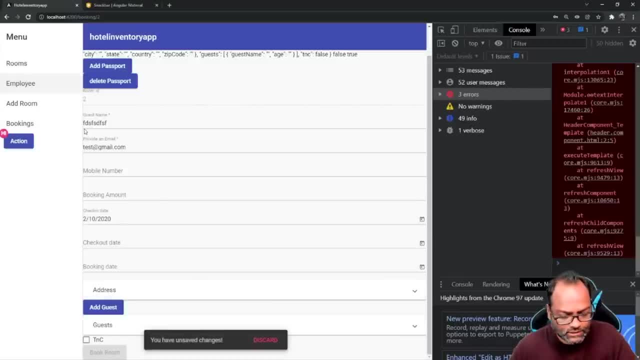 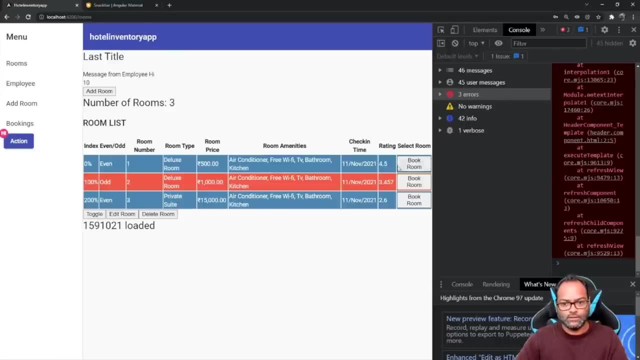 sure that it works. so now let's go ahead and verify this. but it's only standard for our naSer, NOT in appmodules functionality. so you can see, let me just refresh this page. so we go to login admin. and then we logged in, click on book room, go to employee works, go back book employee. now let's make this form. 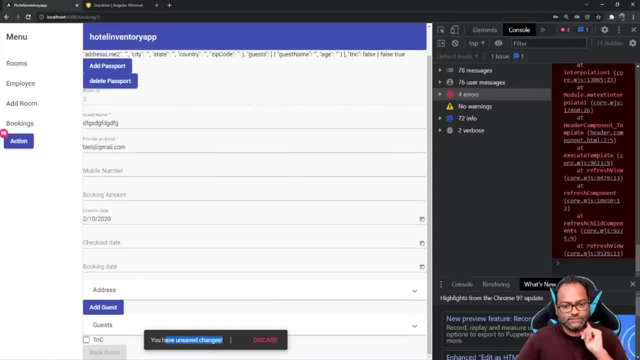 dirty. let's try to move. and you can see you have some unsafe changes, so we are not able to redirect. but we are also displaying this message that you have some unsafe changes and you can just discard, complete the form and then, once your form is in pristine state, you can just go ahead and 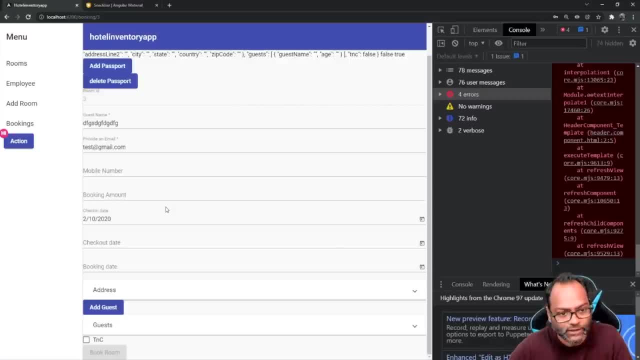 redirect or move from this particular url. so this is how you can uh, use, can deactivate card. this was a real-time example which i can give you. sorry, this was a real-time example which i can give you. you can find more uh, more real-time use cases in your application as you go, but you don't have to. 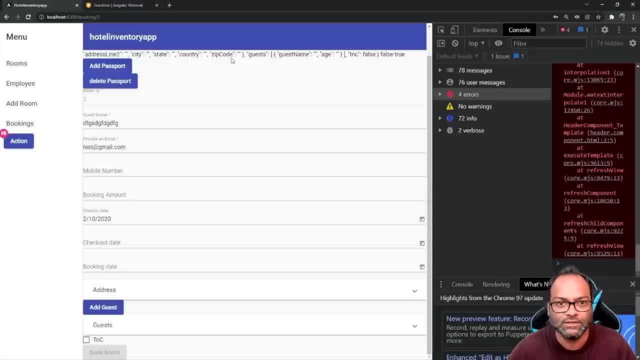 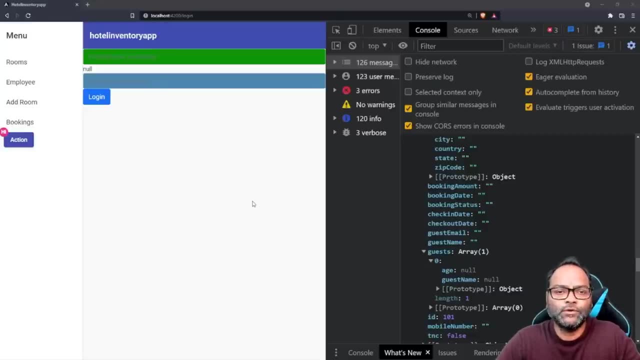 probably you will not get the scenario i mean once you start the application. so yeah, this is it. so now, next, what we are going to do is we are going to discuss about how you can use form control. you might might be wondering: okay, we already saw form group and we also saw form. 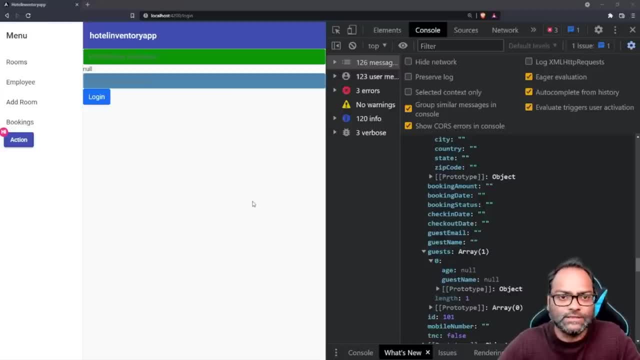 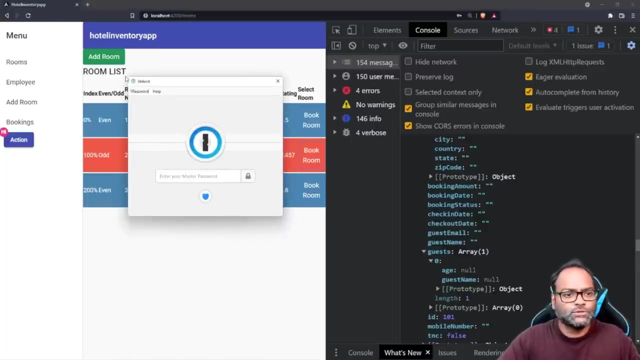 control now why we are talking about form control again. so we'll see that example and we will apply that with a pipe. so we will write our own custom pipe. let's talk about the scenario where we are going to use it. so on this page, right? so if you see this on on this page, what we will do is we will add a text box. 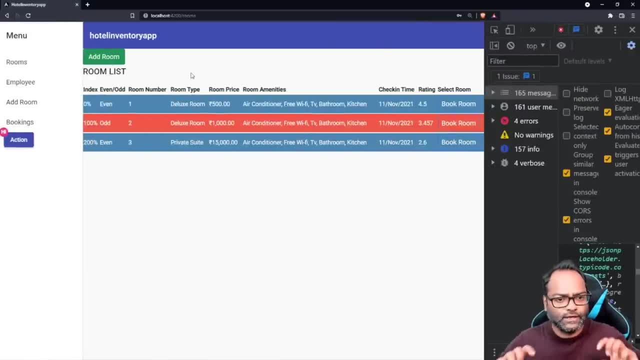 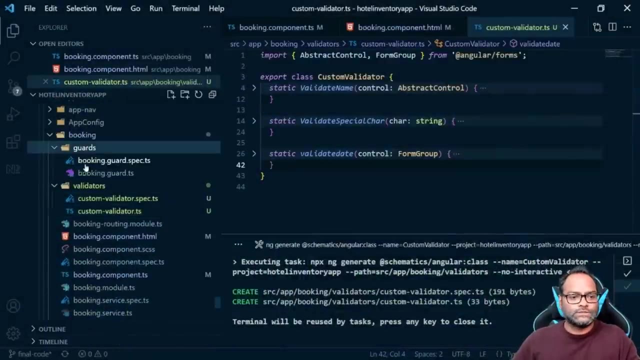 here which will be like kind of filter where we can enter the room price and it will filter the values based on that room price. okay, so let's see how we can uh do that. so this is our rooms page. let's go to the rooms component page. let's go to the rooms component. 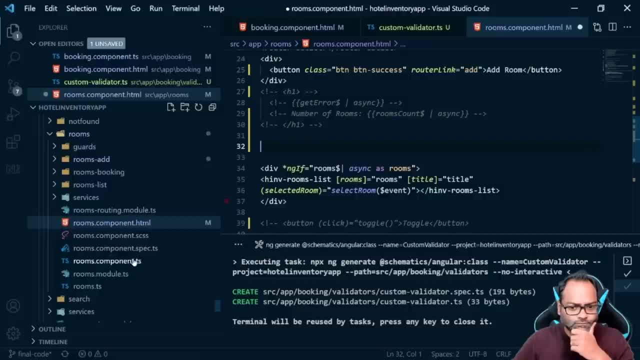 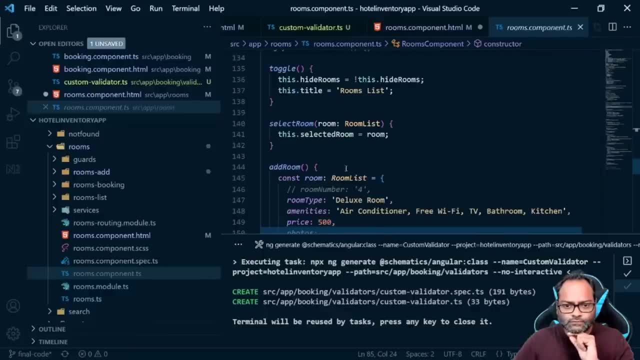 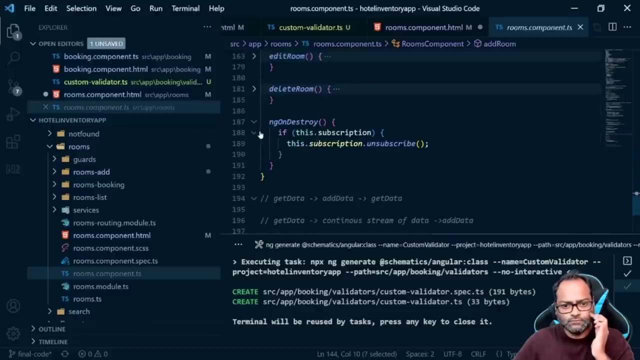 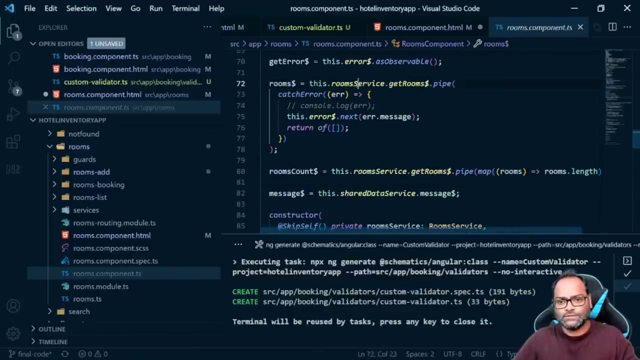 here. so if you, if you remember this, values is actually coming from this particular service. so we are calling room service and from here we are getting this, all these values. so what we will do is we will apply a filter, something like this: so let's, let's, let's. 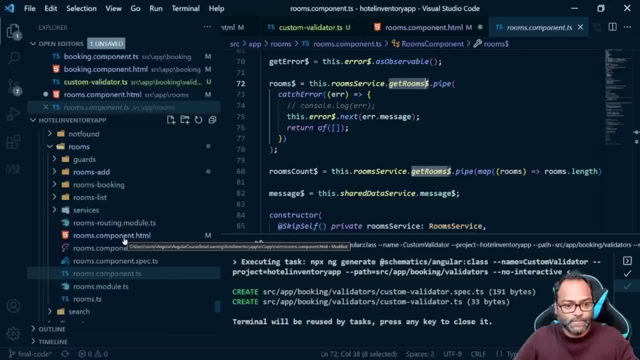 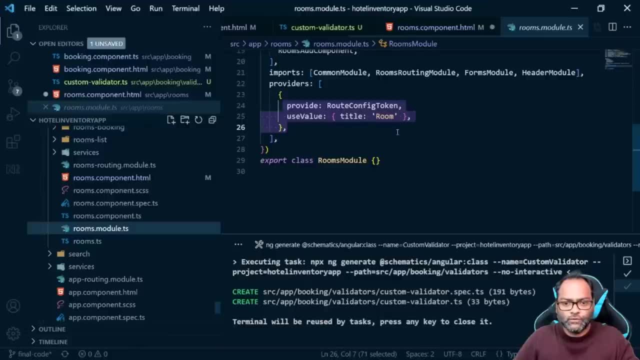 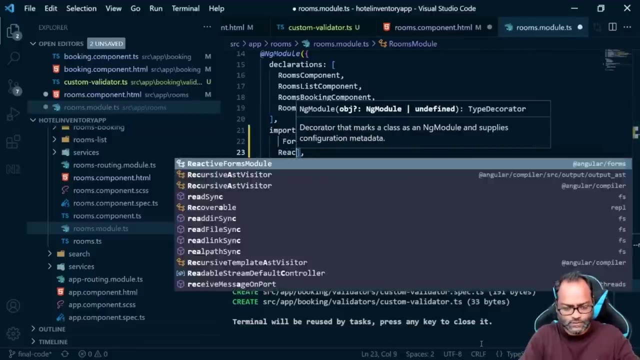 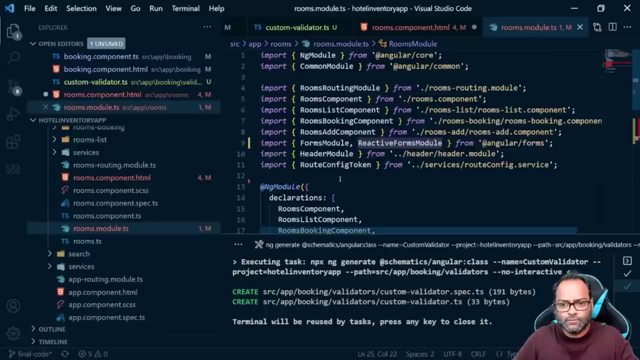 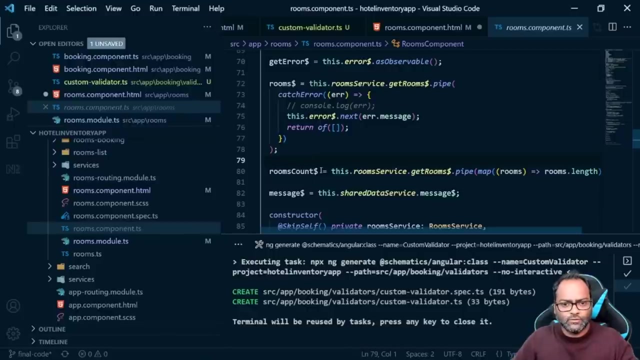 try that out. let's do- uh, let's write the code first. so we are going to use reactive form here, so we will add reactive homes module first and let's create a form- sorry, a form control, because we just need a single control. and to do that, what we will do is we will create- um, we'll call it as a search or price filter. 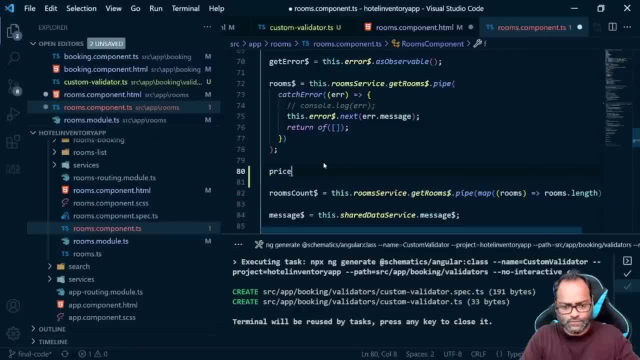 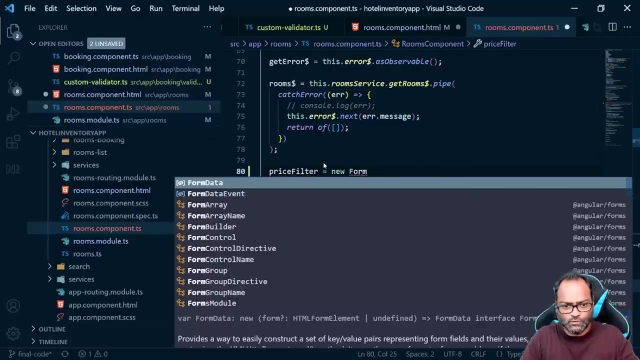 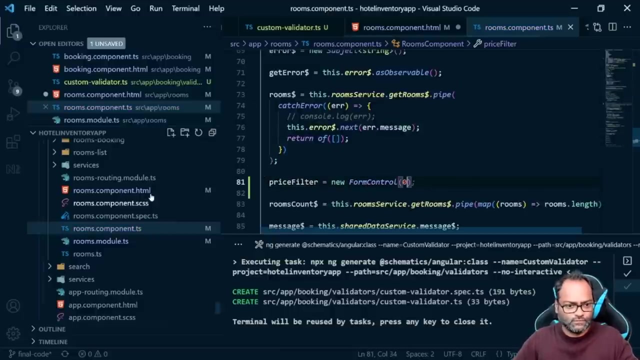 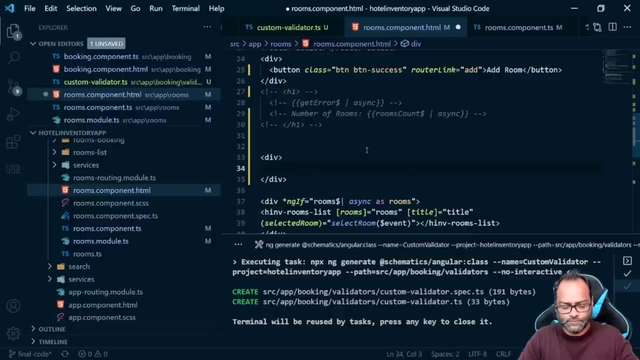 so we will create a search and we will call it as a search or price filter- sorry, which is, is type of or which is equals to new form control. remember this: we are seeing new form control and we are passing default value as zero. let's render this here. we will say: this is div and we will provide our input input type, which will be: 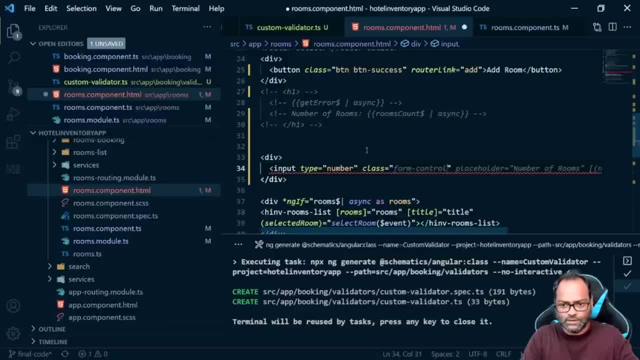 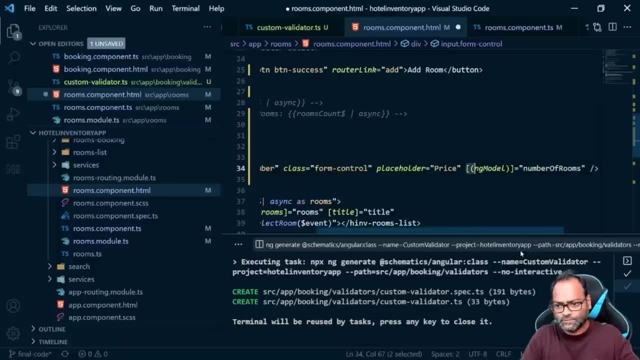 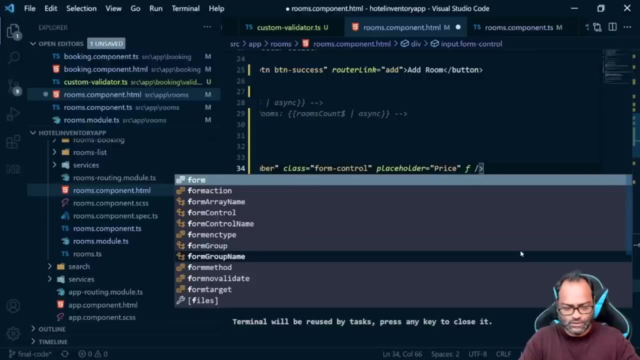 number and we will provide our input type, which will be number, and we will provide our input type, which will be number class, which we'll say is form control place holder. we will say: this is price and here, as we don't have form group, we will be using something known as form. 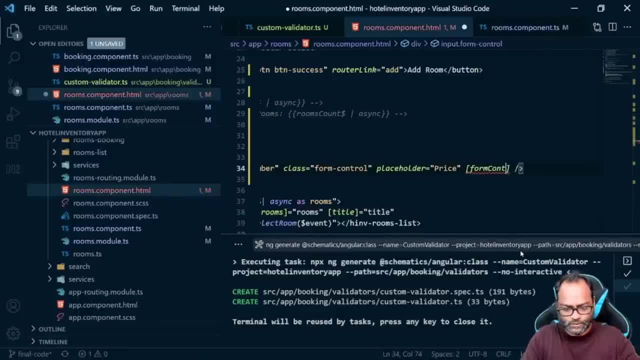 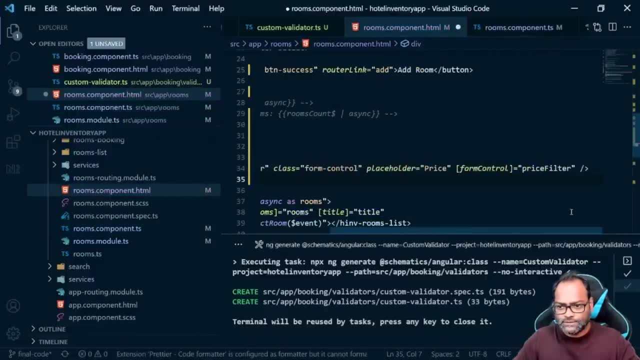 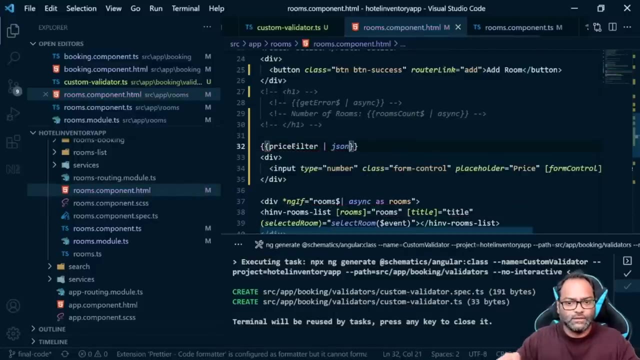 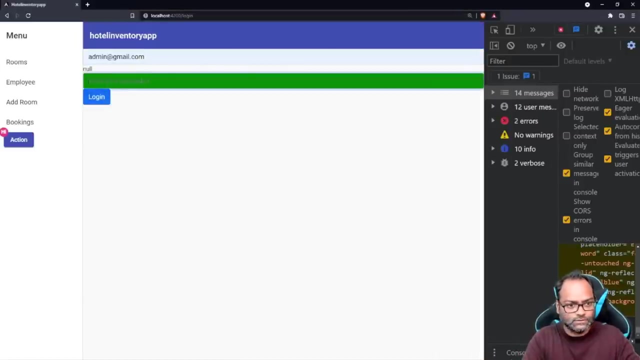 form control is equals to the price filter, and let's do this. so we'll just put price filter here to see if whatever value we enter is getting applied or not. so let's go ahead and test that first and then we'll apply the filter. so we'll. 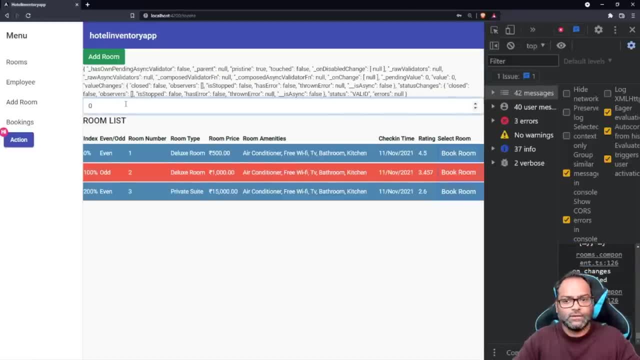 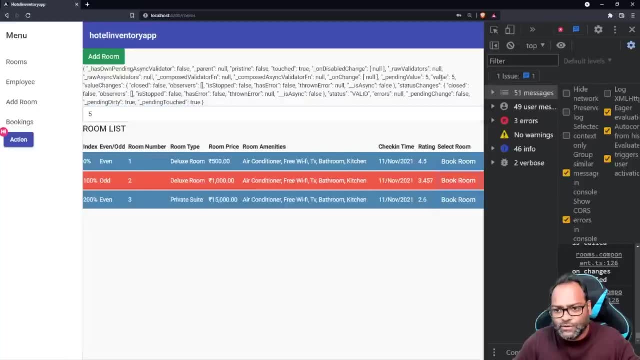 say, okay, this is admin and so, uh, you can see this value right, this value is getting changed. so, as i have already said, the right now it's a control right. so, okay, control will have all the properties, pristine, dirty, all this, all those properties. what we are interested about is value. so value is getting. 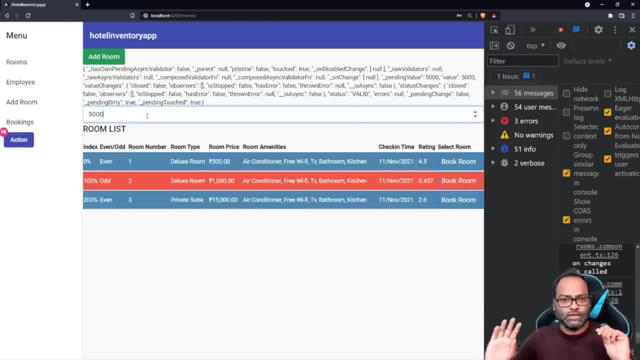 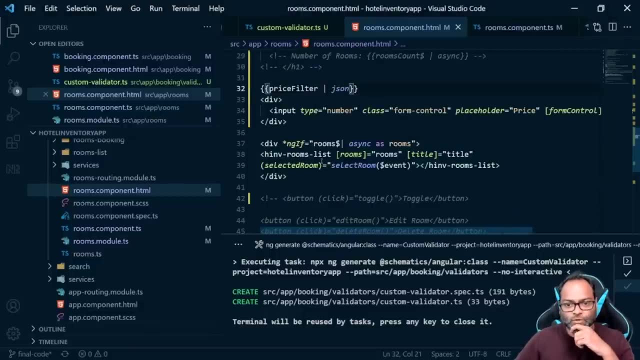 changed. that's it. the first step which we have done is: okay, we are able to apply- oh sorry, we are able to get the values from this particular control, step one- done. now the next step which we want to do is: we want to apply this value filter to this rooms list. how we should do that. 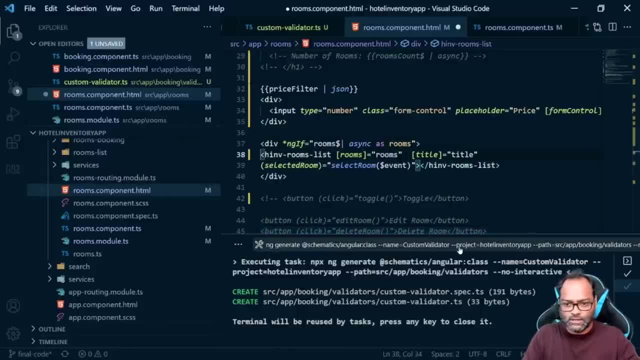 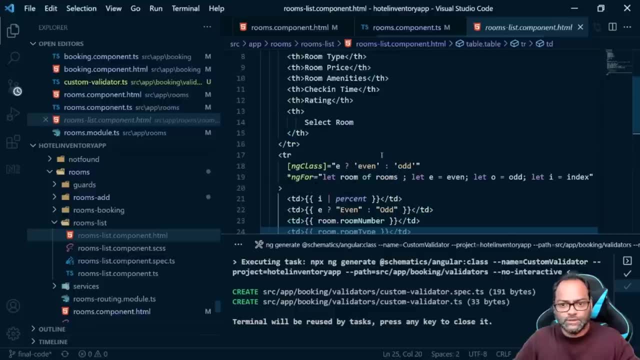 so here what we will do is we will, uh, create another property called price filter. so let's see how we can do that rooms list html and we will apply. we'll pass that value here somewhere with a new pipe which we create. so let's go ahead and create that pipe and 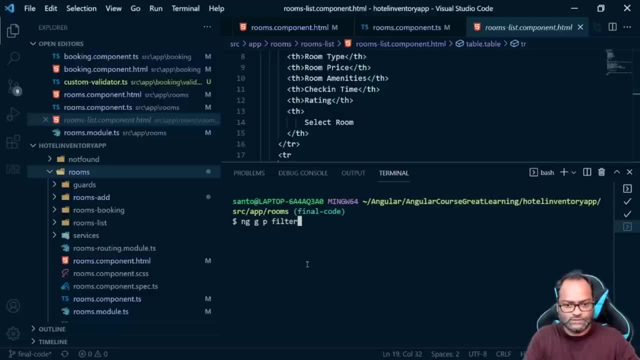 so we can say mtg pipe and we'll say this is filter, so i'm creating kind of a filter. but remember, never do that. no, never do that on a real-time application. always go ahead and do filter sorting at your backend, and i mean at at your api level, just don't do it at your. 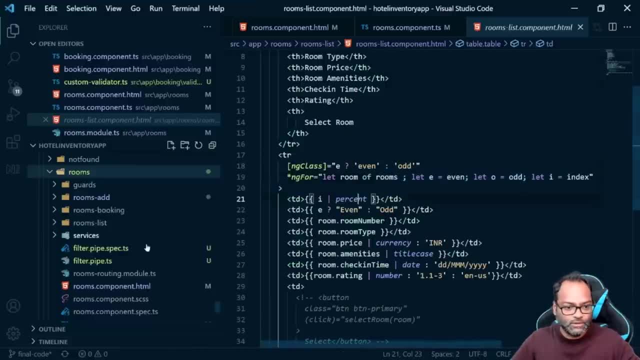 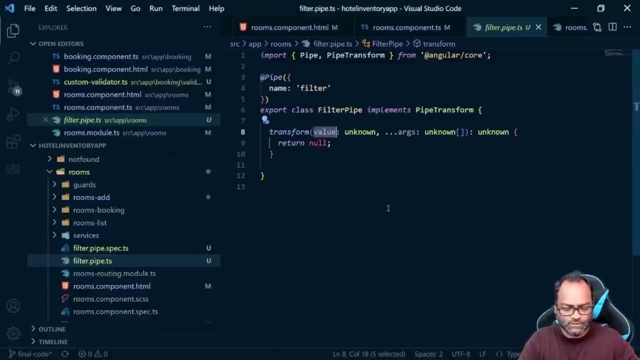 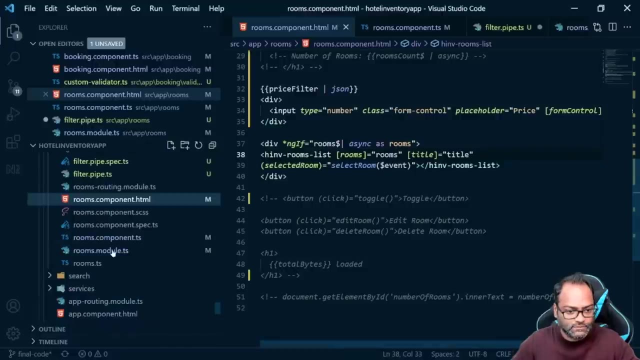 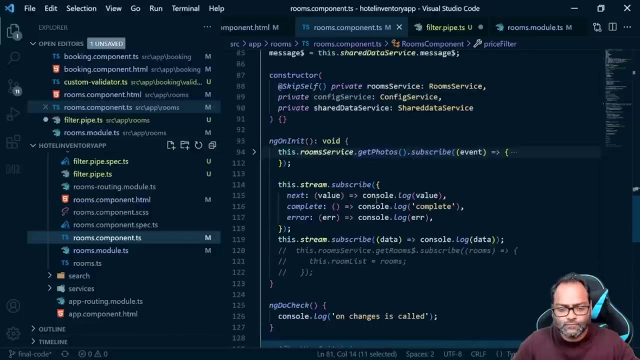 front end. i mean, this is just an example. and now, uh, we can say, okay, this pipe will have multiple parameters. so first parameter is something which will have the list of rooms. so i'll say: this is rooms and which will be of type. let's see the type here. 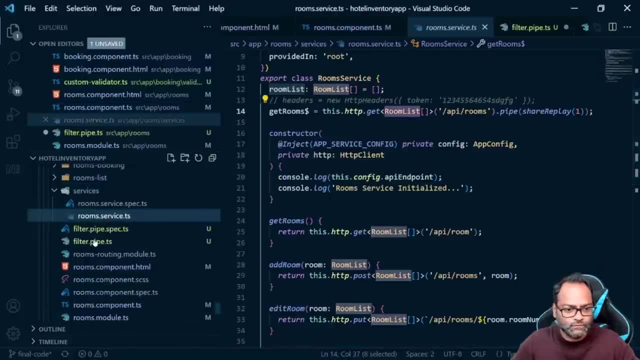 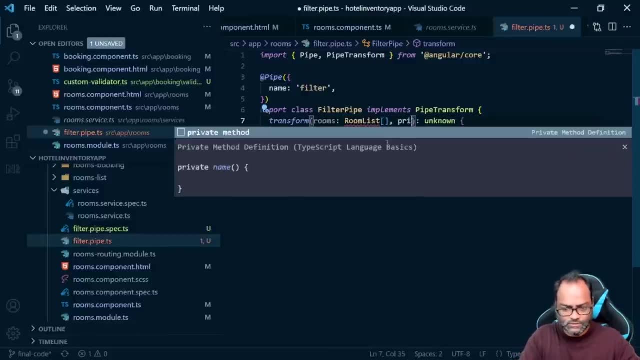 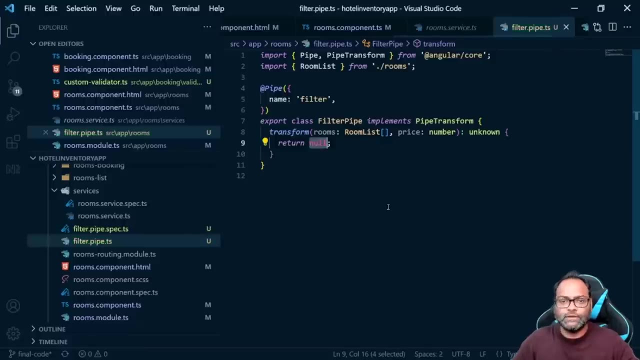 room list, right. so we'll say, okay, this is the array. and the second parameter would be price, which is type of number let's say, and here we will return, we'll say, okay, this rooms dot filter where price is less than this price or, sorry, where rooms dot price is. 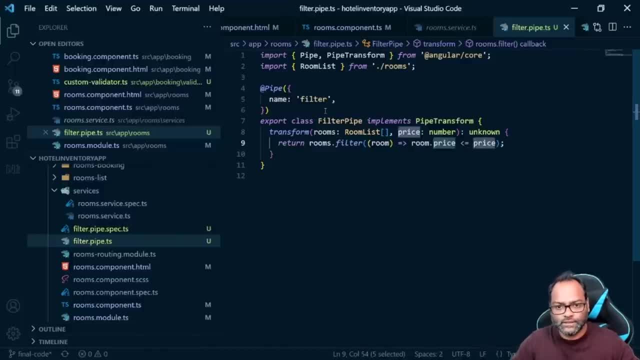 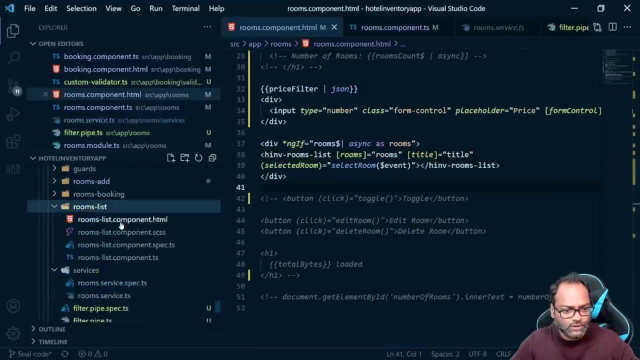 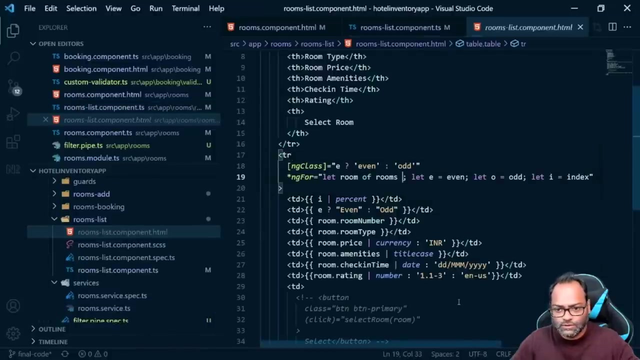 so if we enter 5000, so yeah, it looks correct, and then we can apply this filter pipe. so let's see this rooms list. we'll do one thing- i'll just avoid this change direction strategy on push- and then we can apply this pipe filter and we have to pass a value. so let's pass 1000, right. 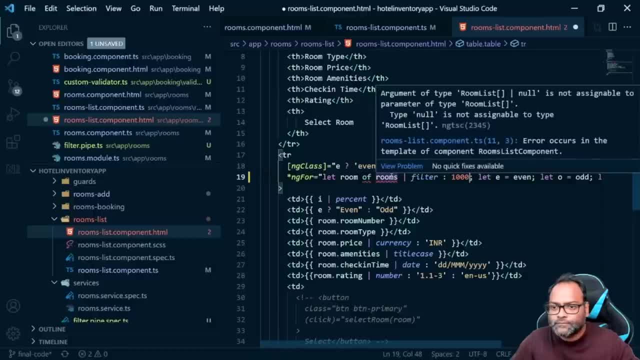 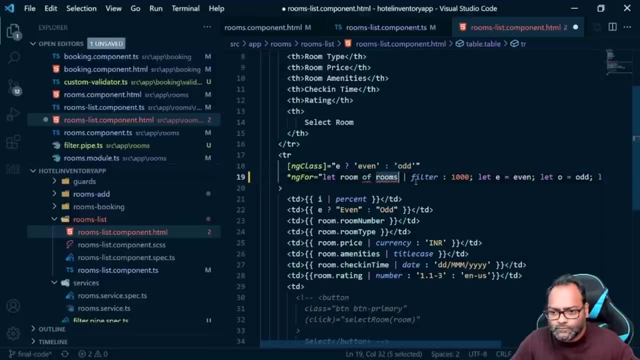 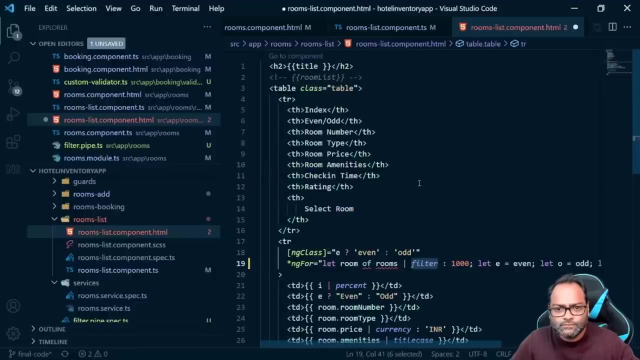 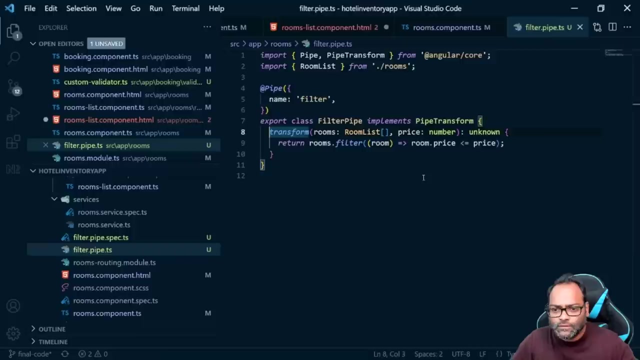 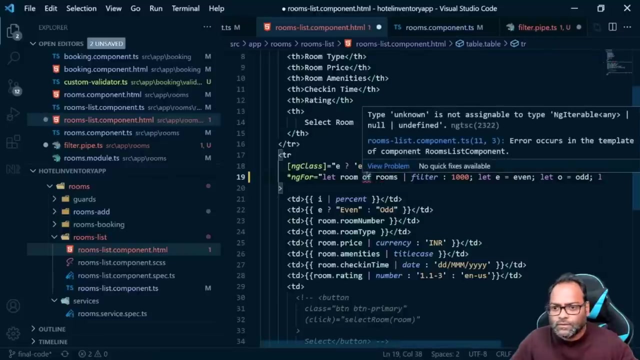 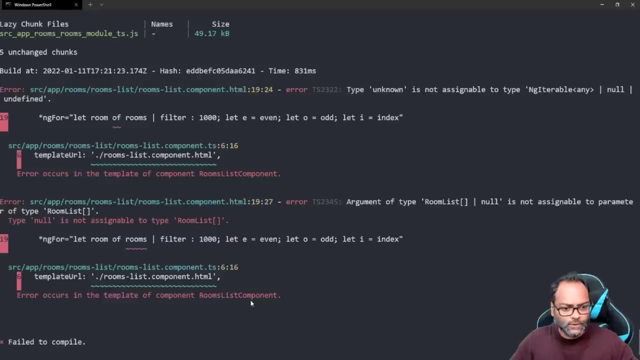 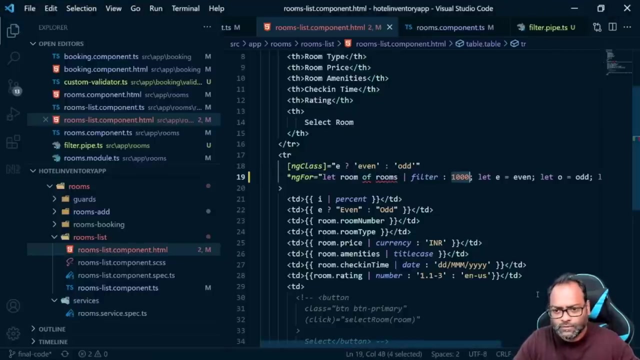 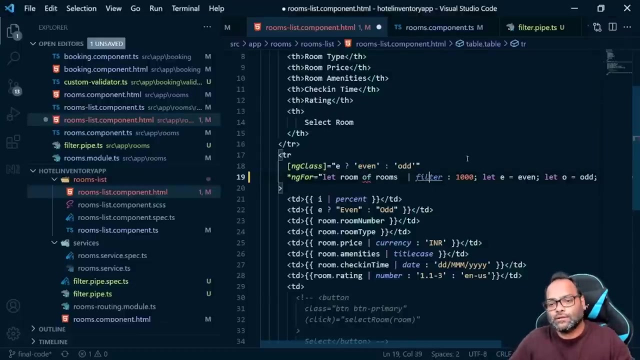 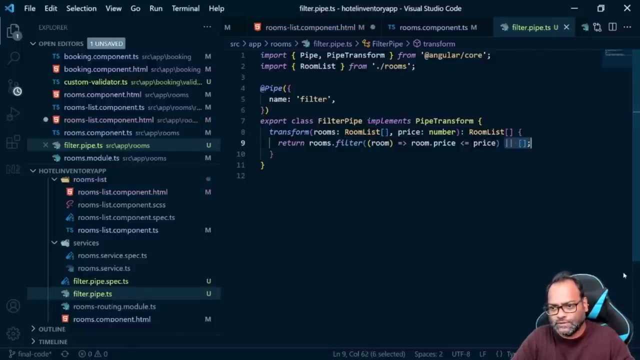 now. so one room of rooms. so okay, let's see, unknown was not assigning you. let's see, let's fix this issue. so it says, uh, unknown, okay, so here, if you remember, we are actually passing unknown here. so we'll say, okay, this will return an array, we can remove this, an empty array, in case. 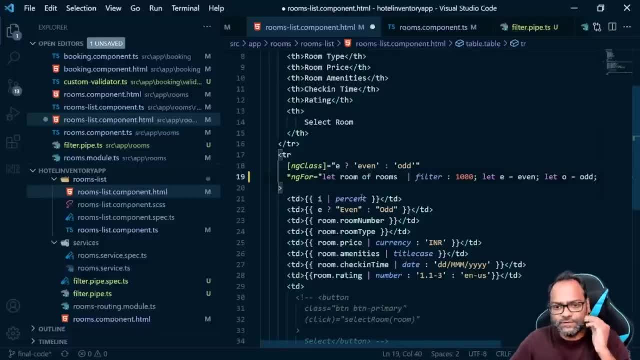 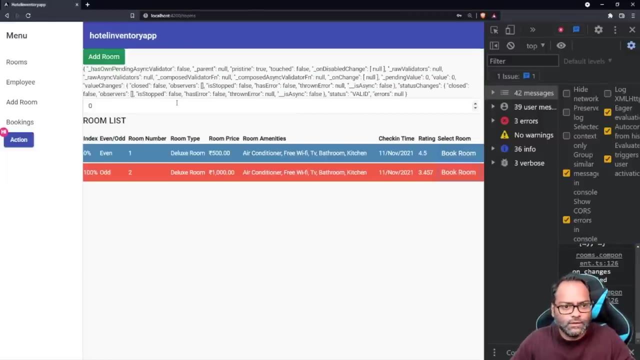 this is. this is not satisfied. so let's go ahead and test this, because it should work. i mean, we are passing hard coding this values, right? so let's go ahead and see our ui and we will say admin, admin, and you can see it only displays the values, which is less than thousand, less than. 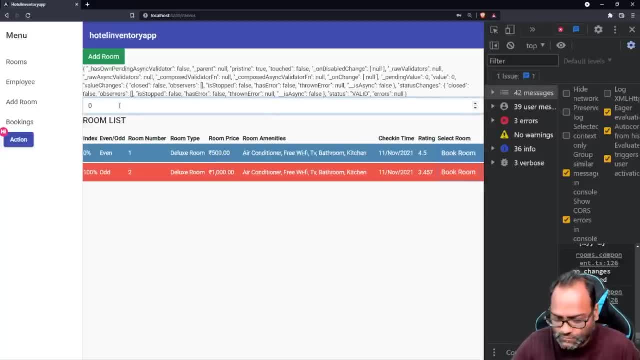 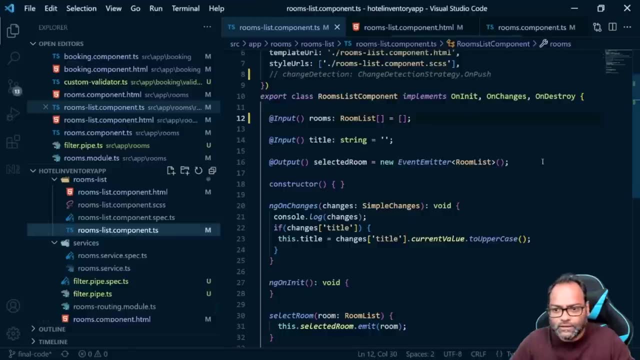 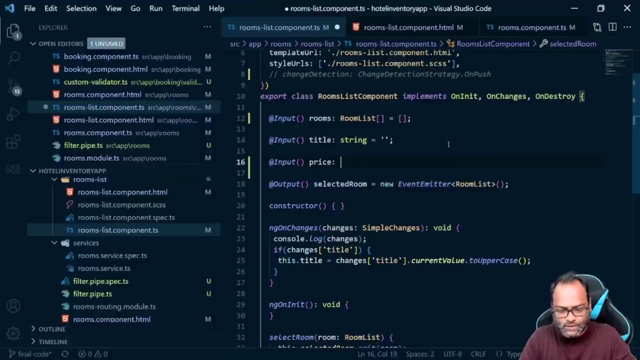 equals to thousand. right now we are not passing this value, so let's go ahead and now fix that. so this value will be our filter. so we will take another input and we'll say: this is price which is equals to zero, and we will use this price here. 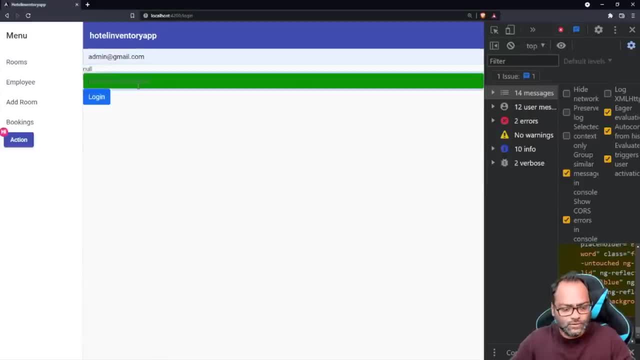 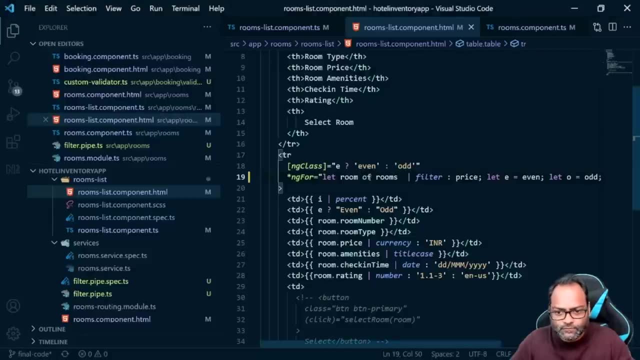 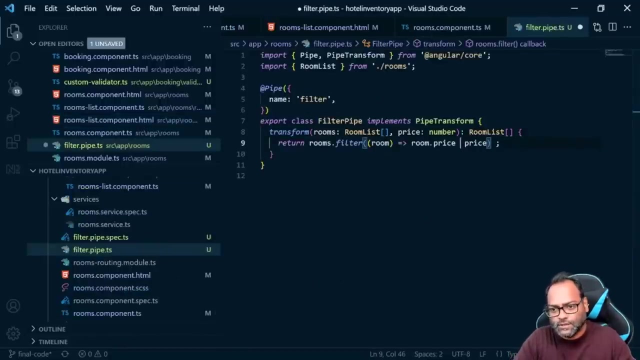 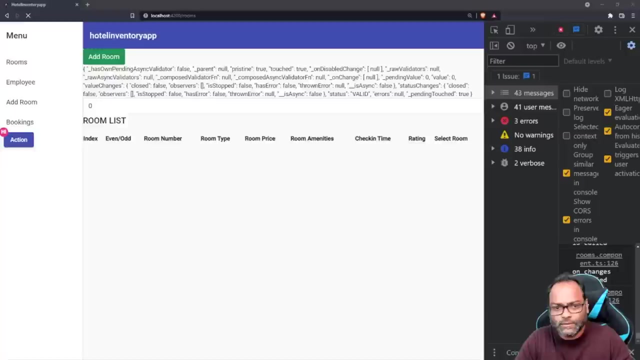 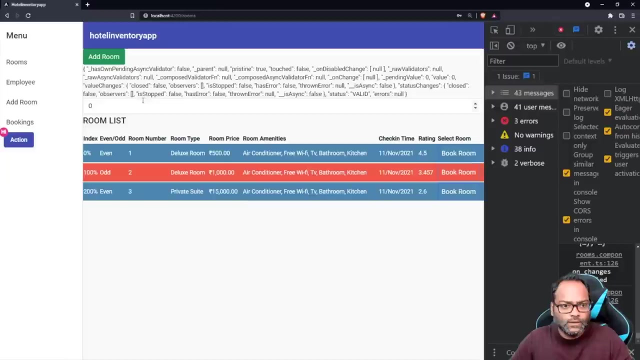 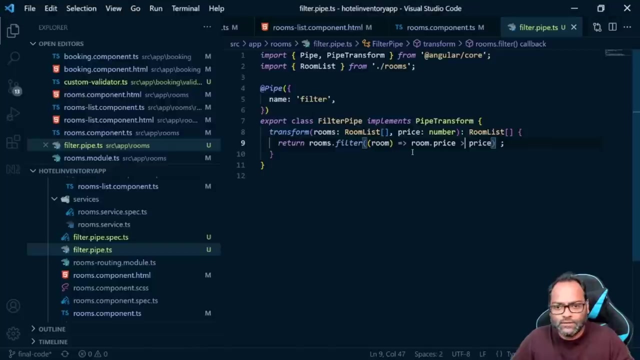 and let's verify again. so and okay, so there is nothing which is less than zero. so i think our filter logic is wrong. we should do this right. so i want to filter everything which is above this particular value. so, yeah, that's, this looks correct, and now let's pass this filter. 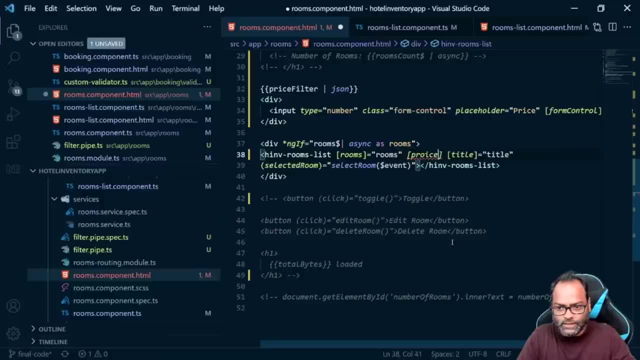 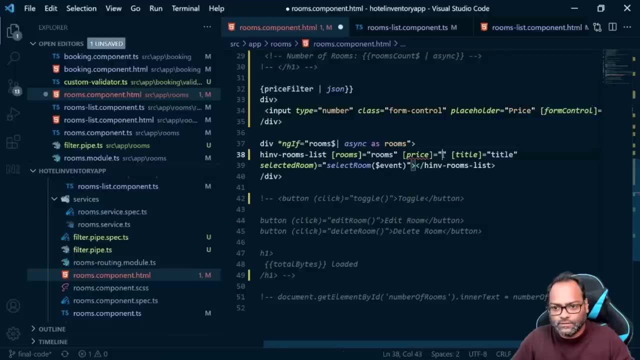 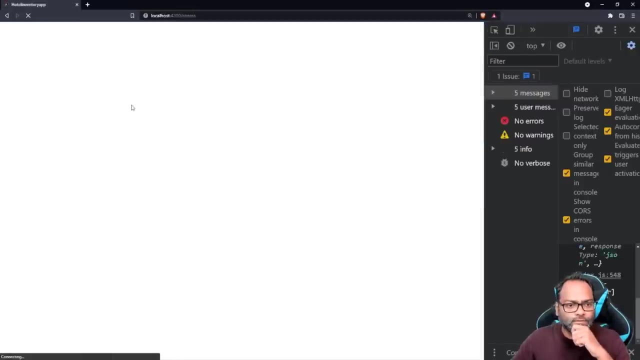 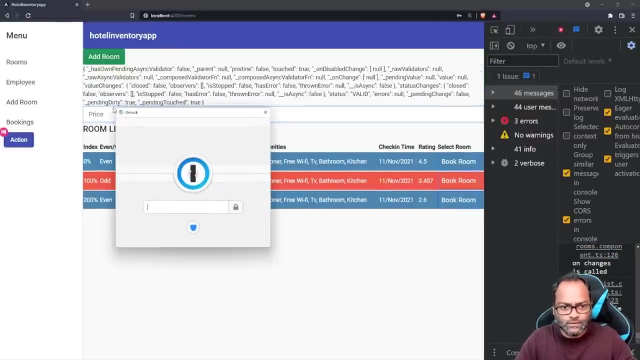 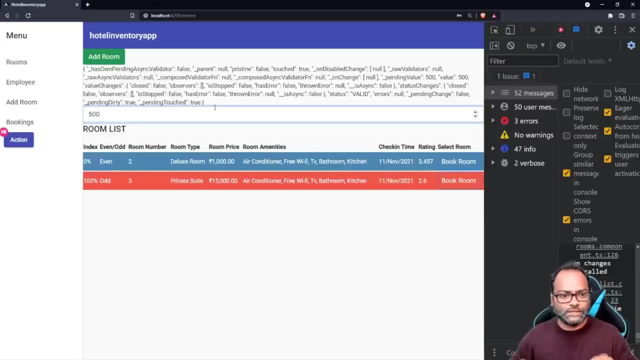 which is now a new, not filtered, but price, which is the new property which we have added, is equals to price. filter dot value. let's see and let's enter 500. so you can see. now i can see only uh values which is greater than 500. 500, let's enter 5000. 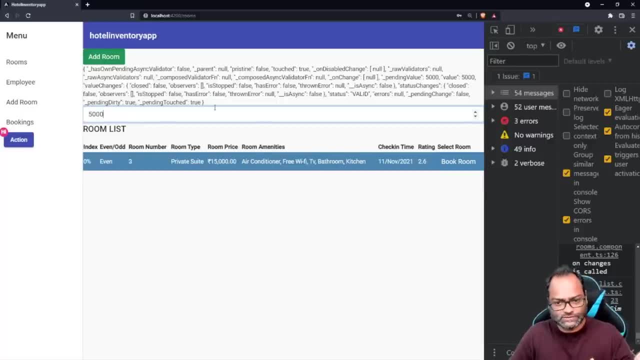 now we can see only values which is greater than 5000, so which is 15. there is only one record which is available. so this is how you can combine form control with a filter. so this is a real-time example which i can, which i can give you and you can utilize it in case of you want to just 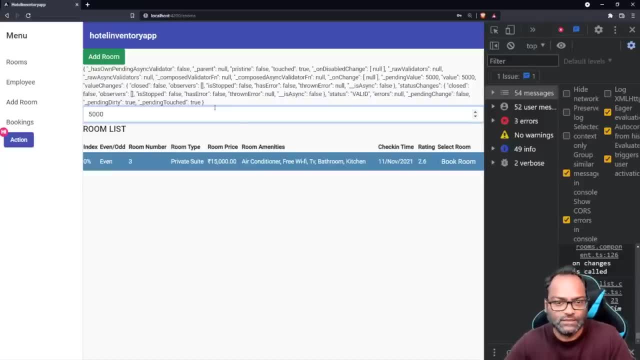 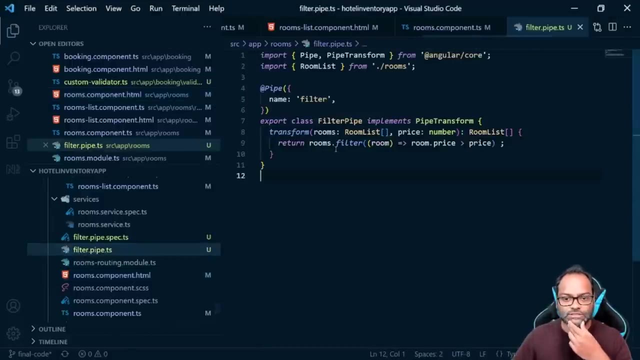 create some filters on your page. you don't want to have a form, basically, so in that case, just utilize the form control, that's it. you don't need to create a form group, so this is the flexibility which reactive forms gives you. and then we applied, we added it with a pipe, custom pipe- where we wrote a logic that, whatever price we provide, 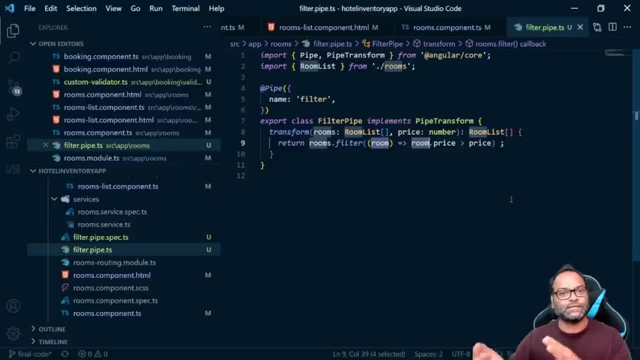 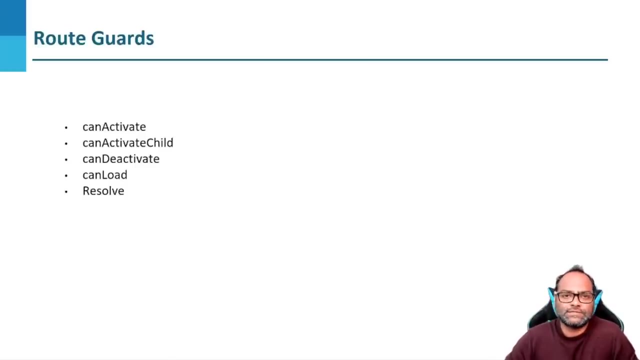 it will filter out all the room plus price which is greater than this price which is provided. so this is it from reactive forms and let's move on now. let's go ahead and talk about the last card which we had left and we said, okay, this card is a little bit different from the existing guards. we saw that okay, can activate. 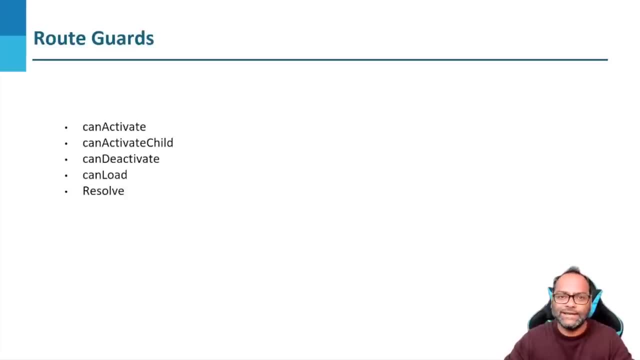 can deactivate, can activate child and can load cards are related to the routes, but what about resolve guard and why it was not available when we tried to create a guard and it was not available in the in the list of options which we had. so resolve guard is actually related to data switching. 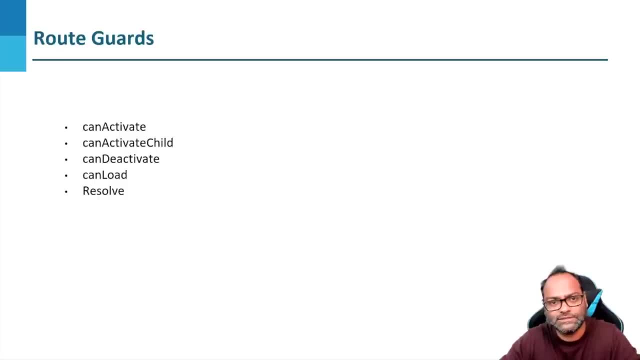 okay, let's see. Let me okay. just. I said data fetching, but it's not data fetching, it's data prefetching. So might be wondering: what is data prefetching? Generally, what we do is whenever we want to display some records or display some data. 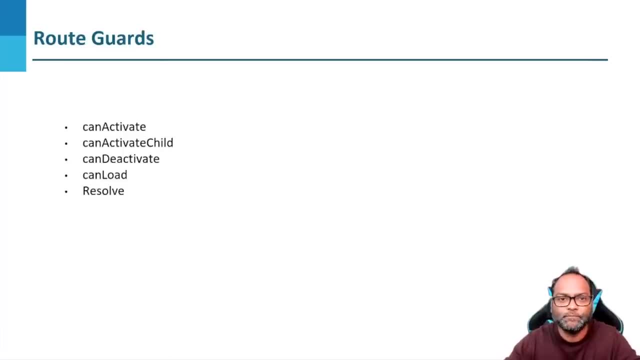 what we do. we go to the component and then we make a service call to get the data. That's what we generally do. But what in case? let's say we have a requirement that, okay, this user should not go to this. 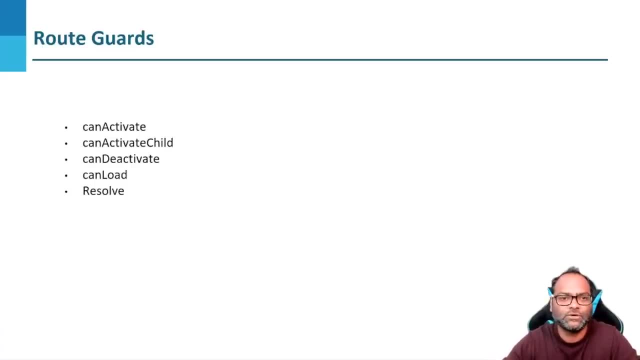 particular view. until and unless the data is available, In case something goes wrong, there is no point actually redirecting the user to that particular view. So this is a scenario where Resolve Guard can help you. So Resolve Guard can help you preface the data. 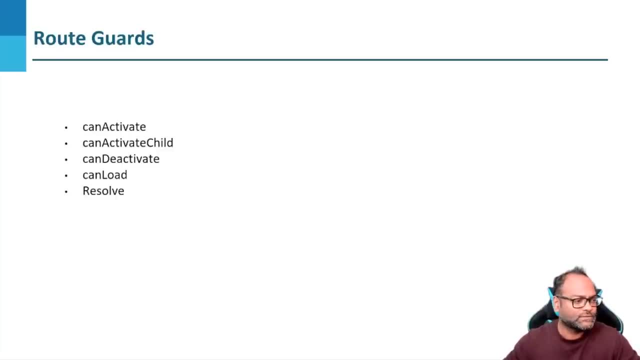 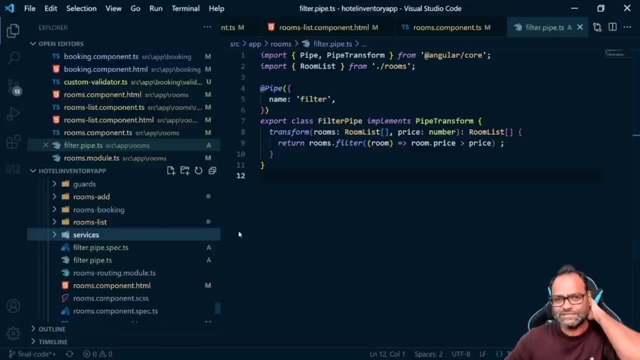 Let me show you an example. We need some records for this and we will be using let's do one thing, we'll create another component and we need some data, So we don't have some dummy data available right now. We need, like more than a thousand records. 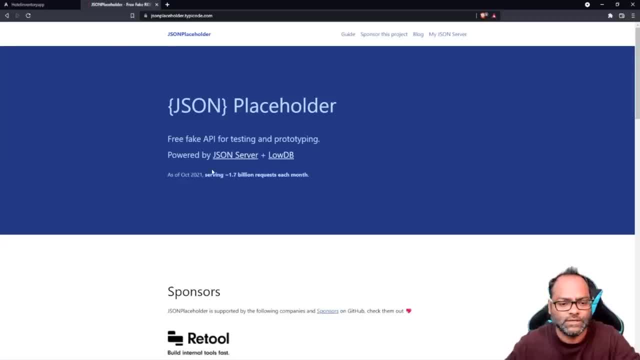 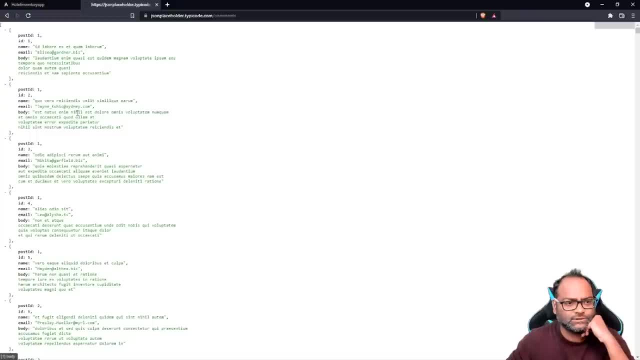 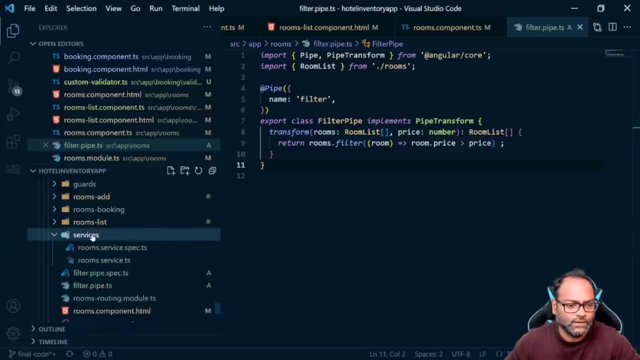 Or let's see how many records this JSON placeholder got. So it has comments, which has like 500 records. Okay, let's see. let's use this comments API and to do that. what we want to do is we want to create another component. 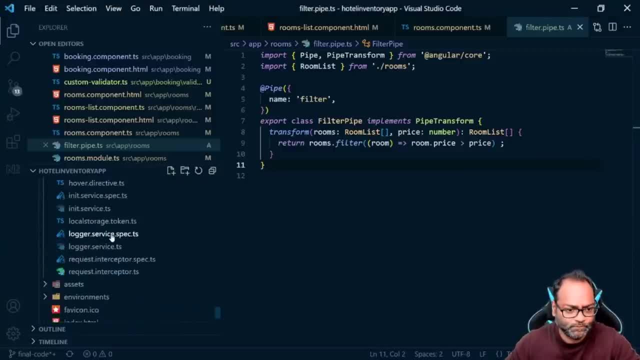 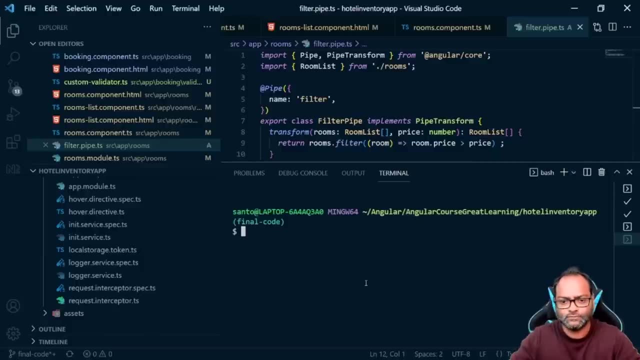 So what we will be doing is we will be creating another component, and let's do so. let's say ng-g-m and this is post. sorry, comment I'll use hyphen. hyphen route is equals to comment and hyphen hyphen routing, and I want. 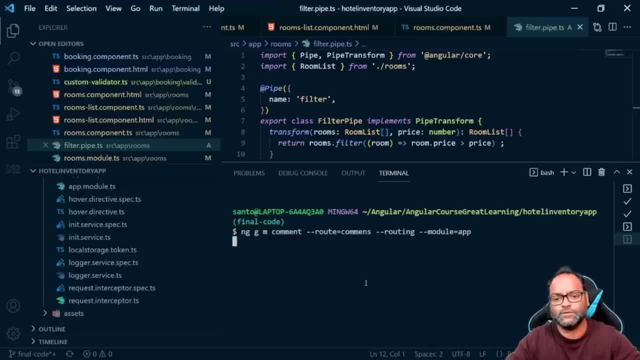 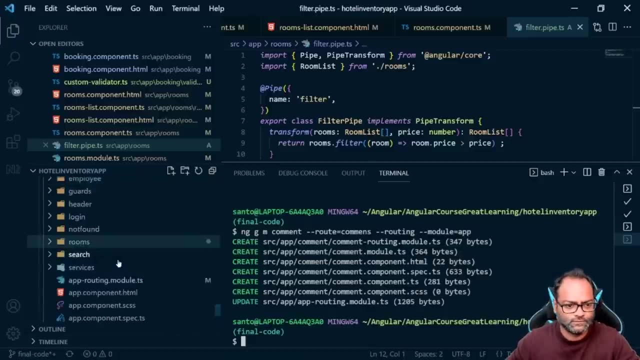 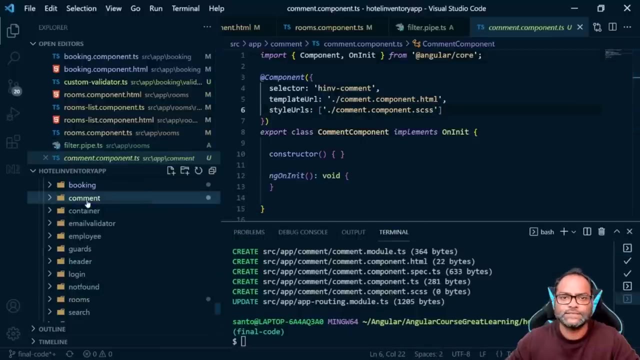 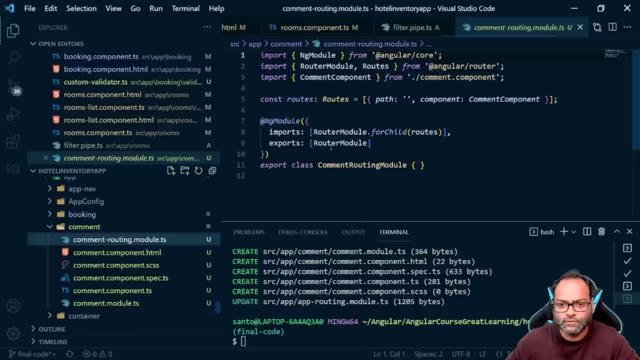 to use app module. I want to register this, So this will be lazy loaded, of course, and we got this component and now what we'll do is we'll create a service for this and let's verify the routing, So we have our route available here and, okay, everything is good. 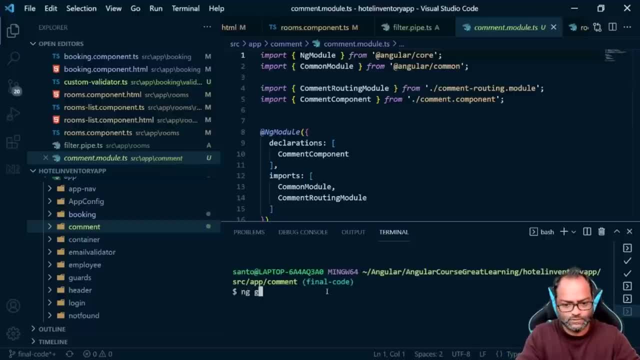 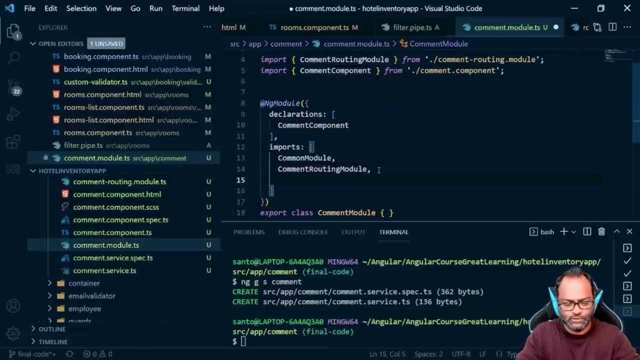 Now let's go ahead and create the service, Okay, so let's go ahead, and let's go ahead and pull up ng-g-s, and then this is comments service. We are going to need http-client module here, as we are going to make an HTTP call. 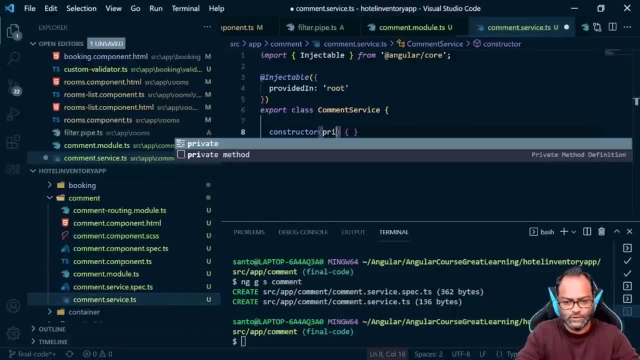 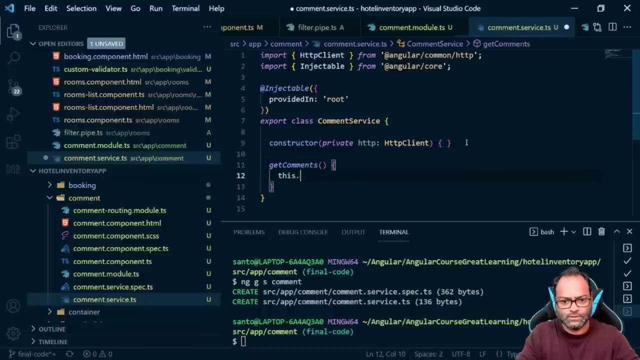 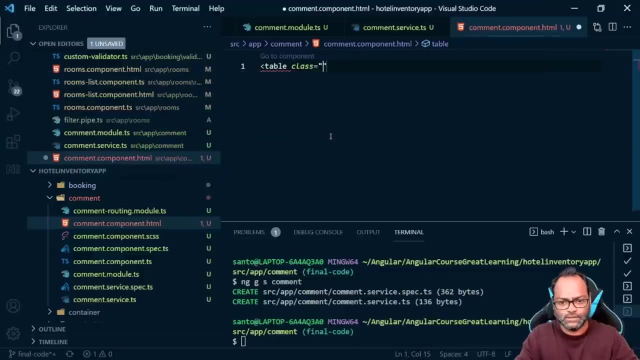 In service. let's inject so its private and end server um http http link and we'll call: get comments, this dot http dot, get and written: this is the api. so we'll use this done and let's, uh, do one thing. i'll just work this and let's create a table and it's a class. 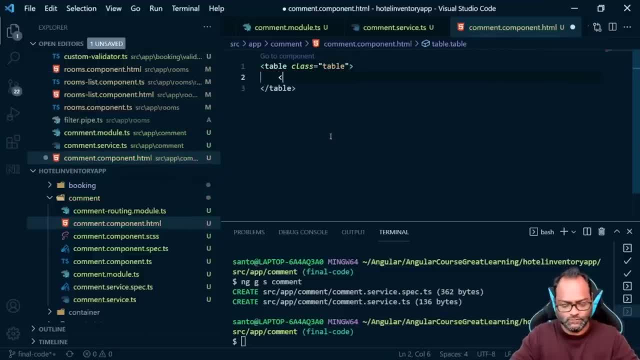 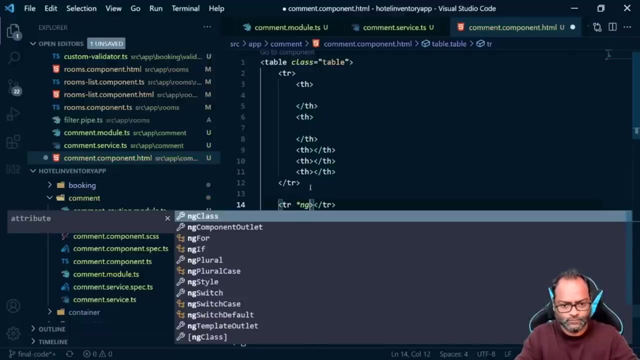 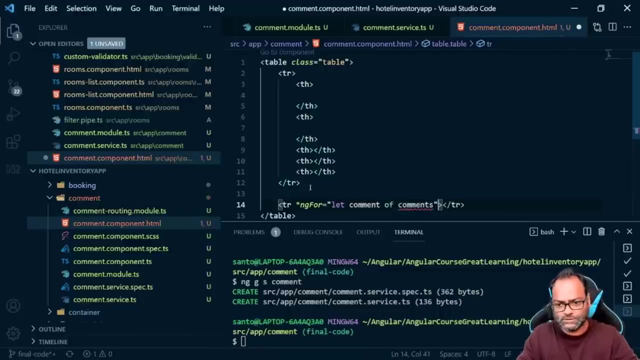 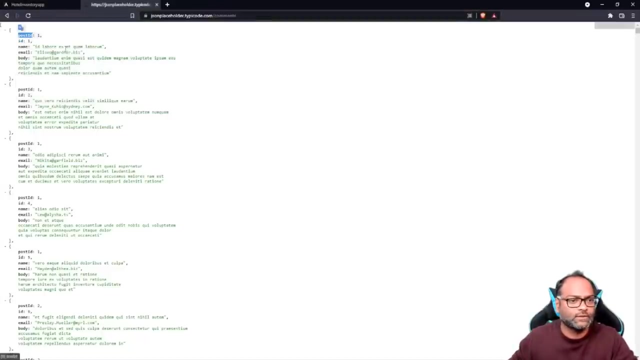 is table and then we will have er where we will put our headers. so we'll have bunch of th. so i'll say this is let comment, talk comments. this is the property which we are going to use and then we'll use some dds. okay, let's see how many properties we got: post id, id name: one, three, four, five. so let's go ahead. 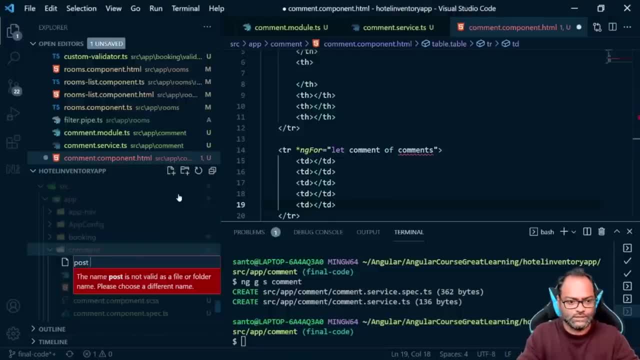 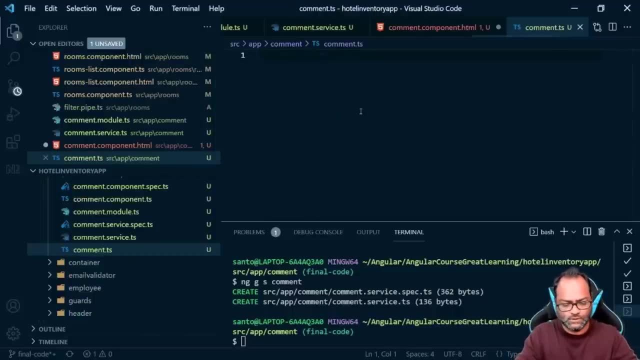 and create an interface. i'll call this as comment: dot ds and let's create export interface number. we have id, which was of type number, post id, which is the gain type of number. i is capital place. we have name, which is string. we have email, which is again string, and then we have a body. 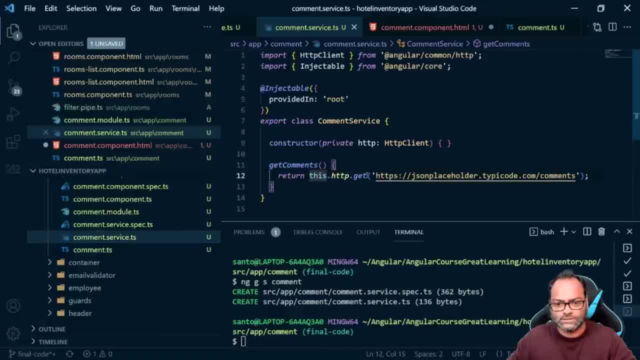 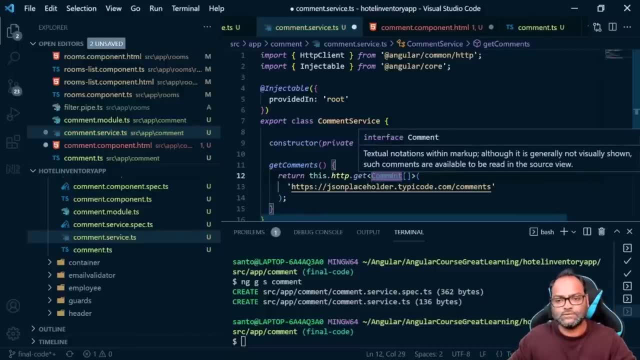 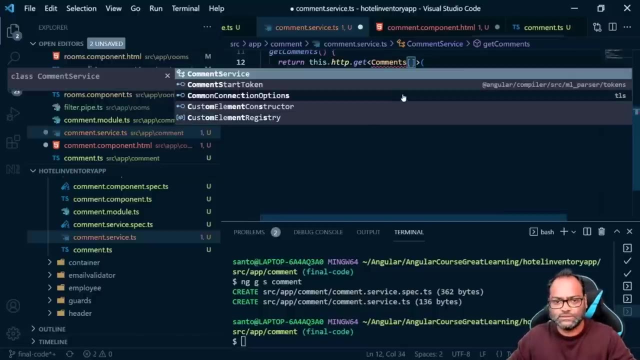 ego, which is again string. let's go to service and say: okay, this, This http get should return the comment array And this comment. remember, there is somehow. there is an comment API which exists inside, inside TypeScript itself, So let's name it as comments, just to avoid this issue which I faced in one of my project. 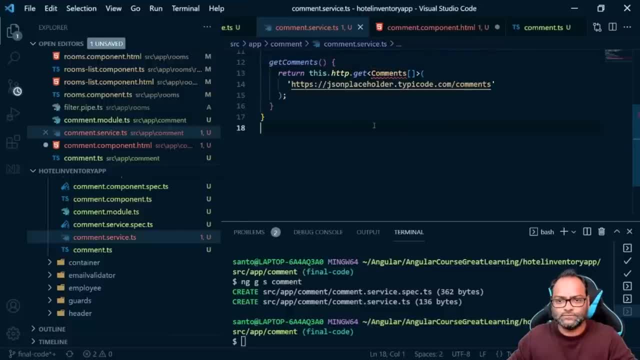 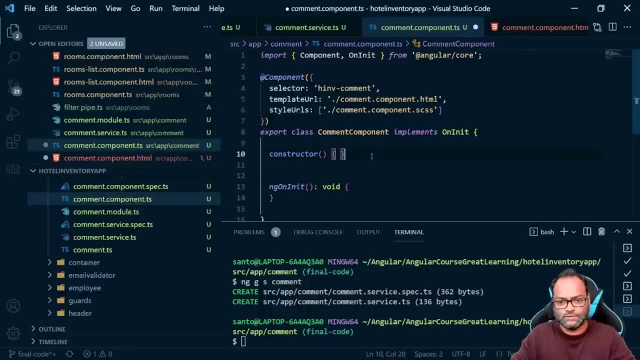 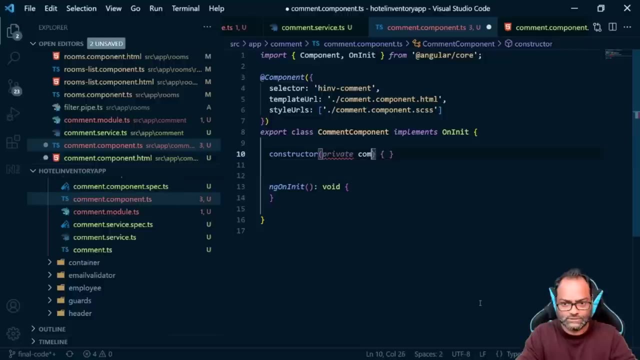 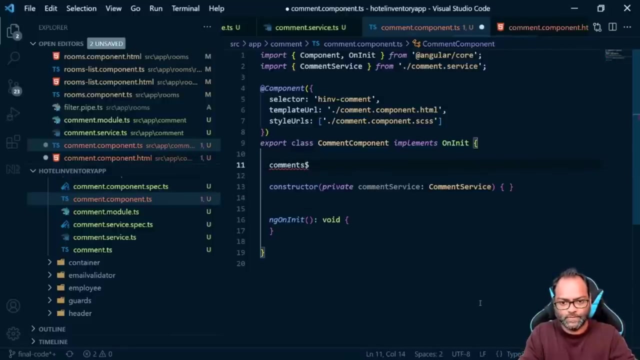 actually, And let's go to component, and here we will use the service, such a private excuse this, and we'll say this is comment service, this type of comment service- And then we can just say this is comments- is equals to this: dot Get comments. 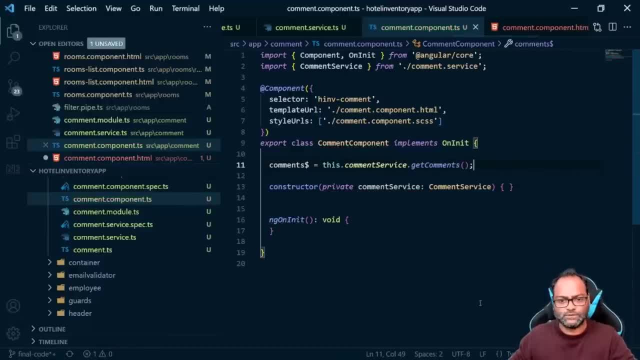 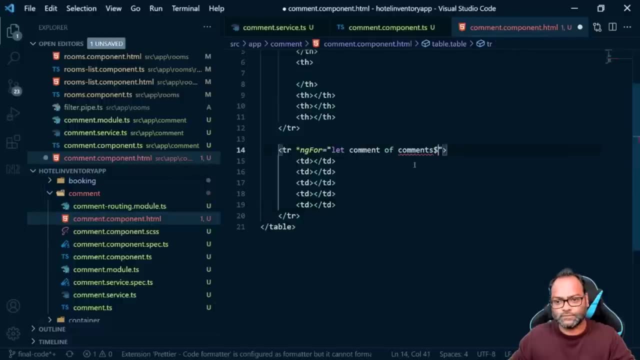 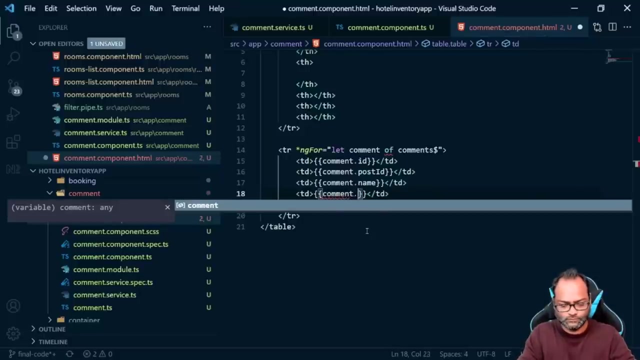 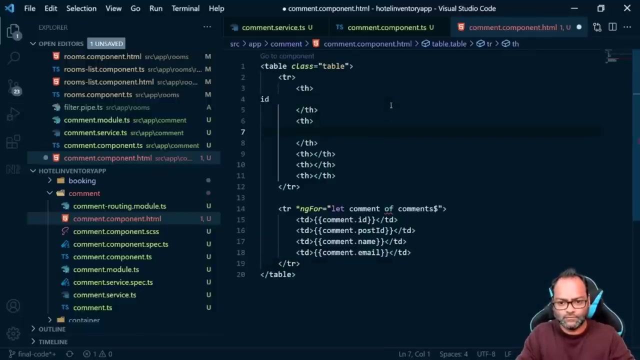 Okay, So now we can use it here with a sync by, and let's use comment dot ID, post ID and we had name, So Okay, Okay, Okay, Okay, Okay, Okay, Okay. So let's use a command dot name, and then we have email. 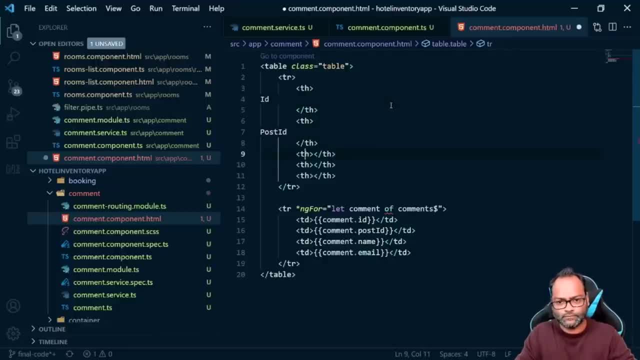 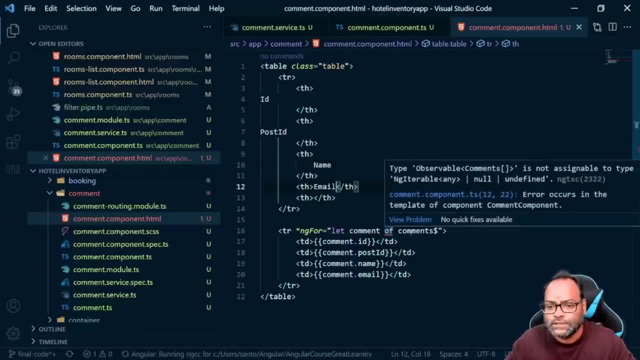 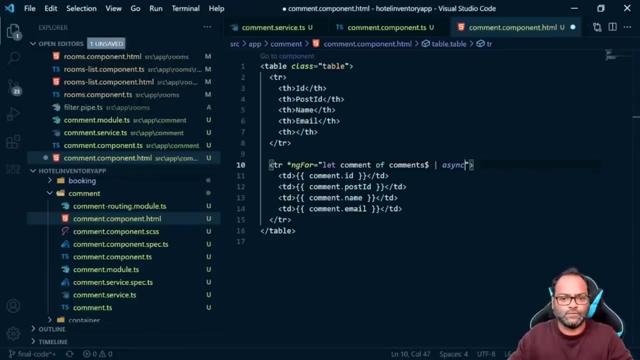 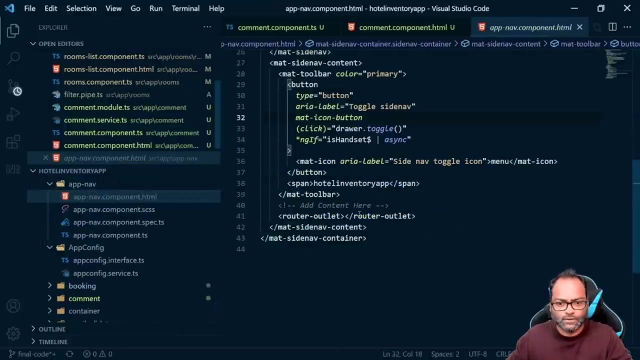 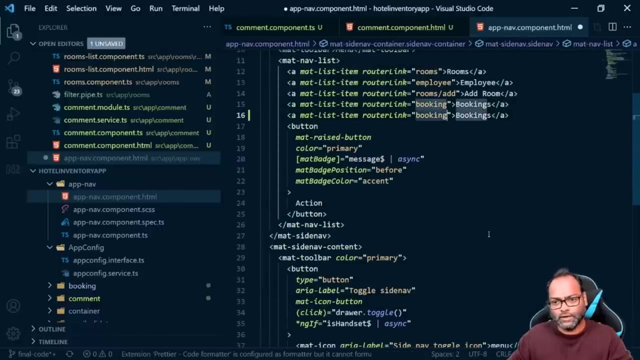 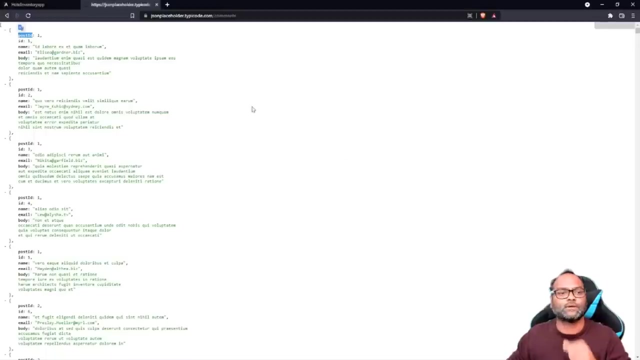 And it's not good body here. It says okay, so we are missing five, a sync, and let's format this format and let's add a navigation here and we will not apply any guard. And this is comment. Let's go ahead and see. 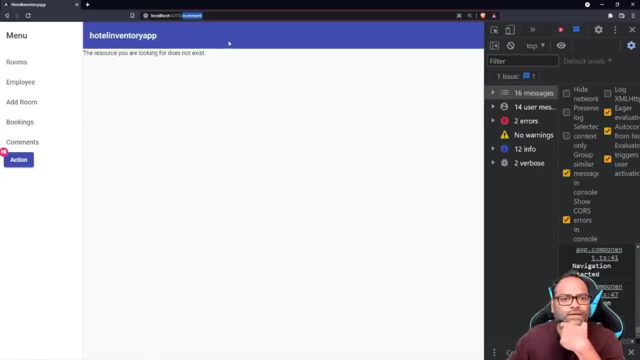 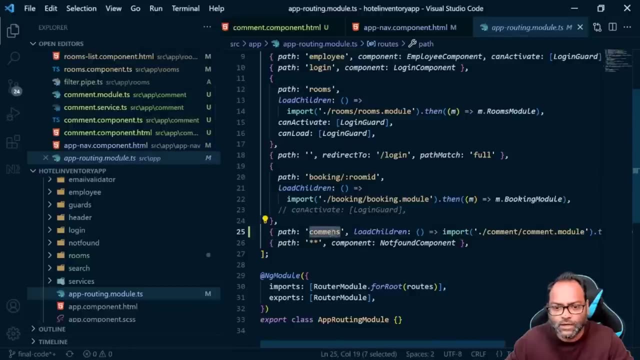 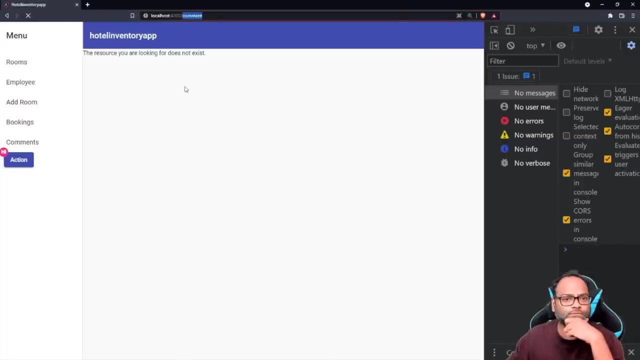 So we have comments available here and it says this is not available. Comment is not available. Why so? Ah, okay, I made a spelling mistake somehow: Comment, Okay, So let's go ahead. Let's see one thing, Let's see a behavior here. 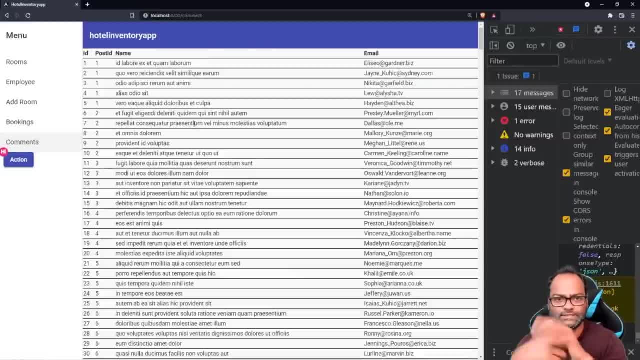 So you can see, when I click on comments, there is an empty page and then the data is getting loaded. So what in case? uh, I don't want to show an empty page, So this is also one scenario where you can actually use it. that okay, when my view is: 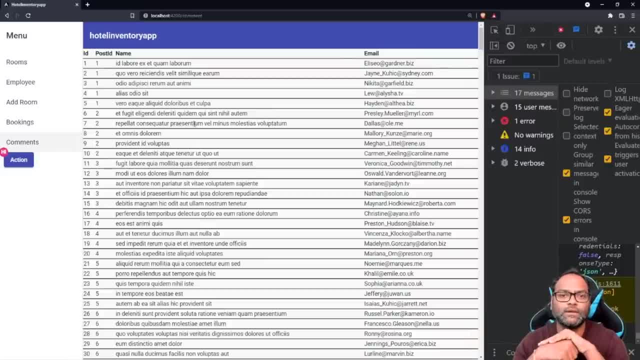 loaded. it should be loaded with data, not without data. But remember, keep one thing in your mind: You can use resolve card with uh use case, where your data will not change after it is loaded. Okay, So now let's try to fix this issue by using the resolve card. 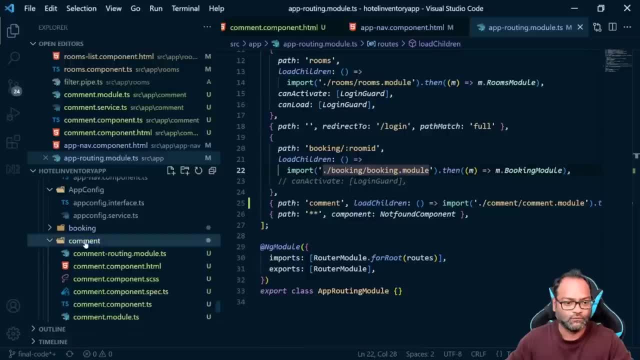 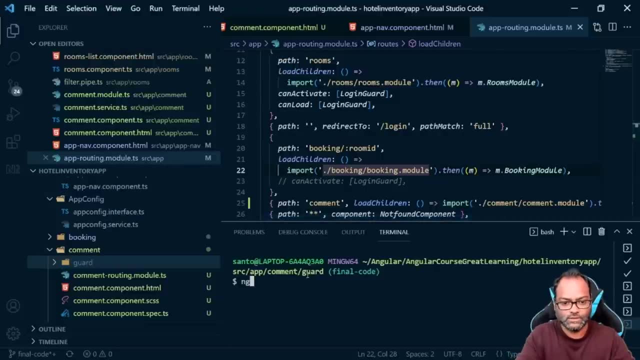 So we will create a new uh folder here. We'll call it as guard. Let's go to integrate terminal. I'll say g, g And this is comment Comment: guard. Okay, So let's, and you can see I don't have any option. 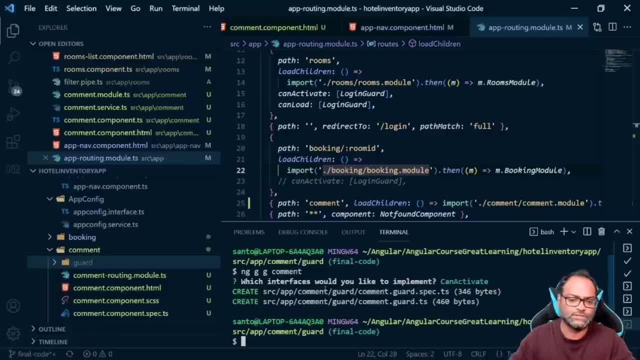 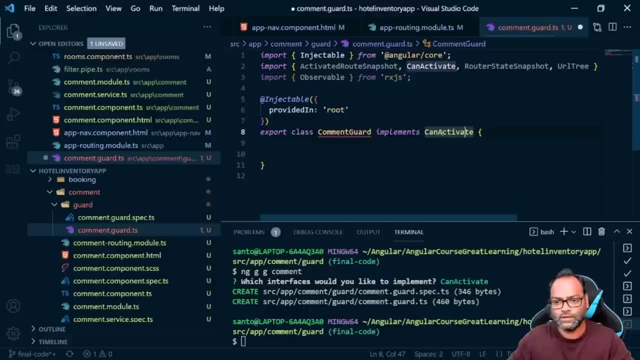 Uh, so I have to, uh, at least choose one. So we'll use, can activate, but we'll remove it. and then let's remove this one and we need resolve card. So this is- I think this is the one- yet resolve, resolve that, and we have to define what kind. 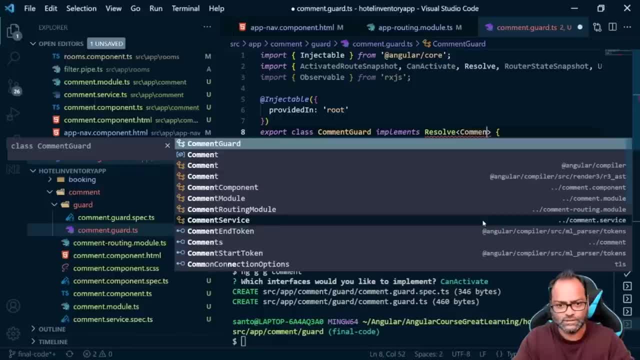 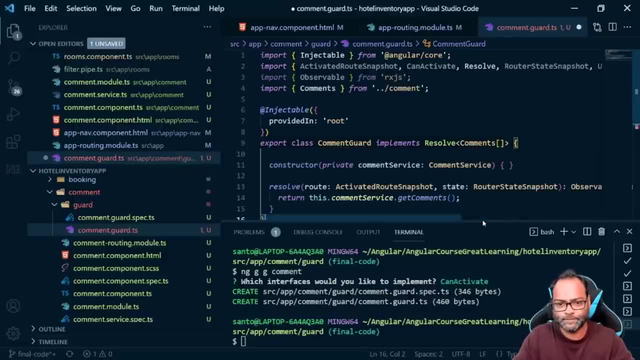 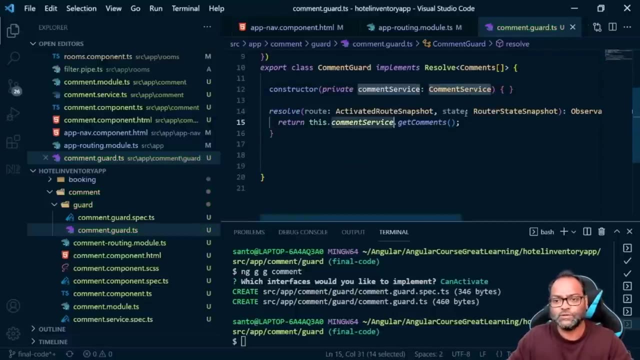 of data this resolve, that will return. So we will say, okay, this will return the comments. Okay, So here, here, here and here, Let's see there's an extra, okay. So you can see right now what I'm saying is: it will uh return, uh. Value of observable. 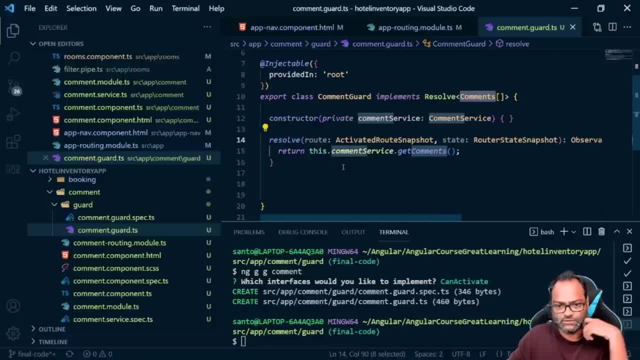 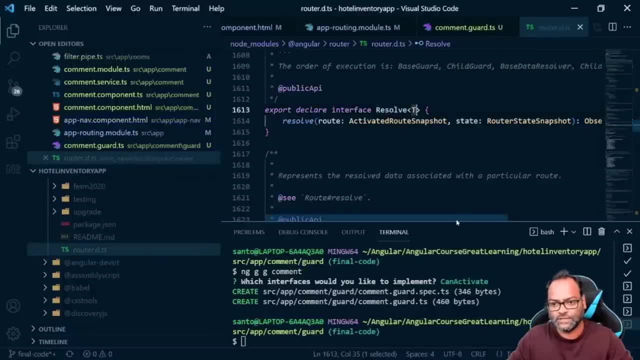 of type, comments or promise of comments, or comments. So we are saying: this is all interfaces, which is coming from here. Okay, So there's all of type D, So which type of data you want done so, comments of array. and this is it. now let's go ahead and apply this comment guard. 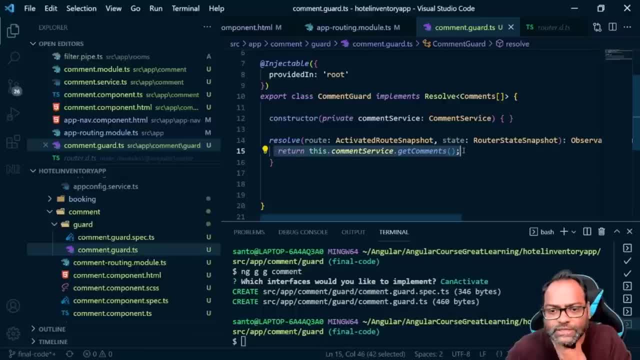 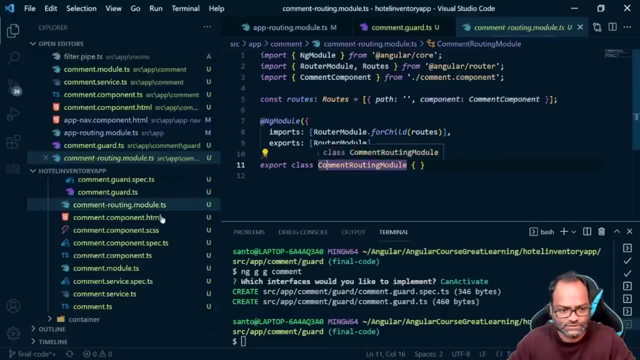 and see how it is. so you can see, i'm just calling the same comment service which which we were calling from the component earlier. so let's go and apply this guard first. so how we can do that, we can go to the guard and we can say: resolve, now resolve. the way a resolve works is it. 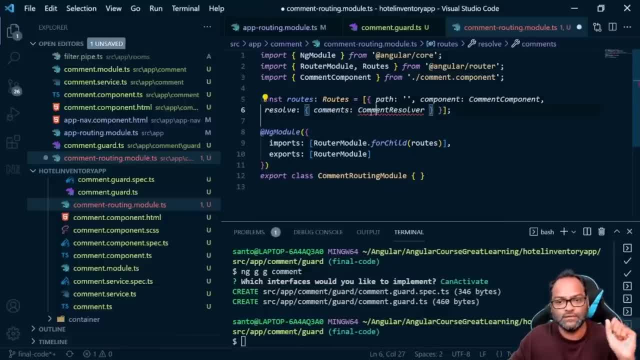 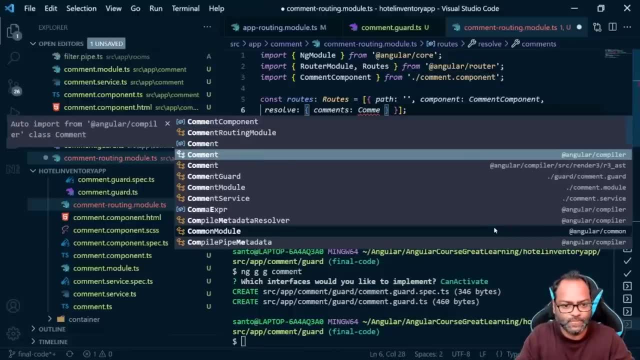 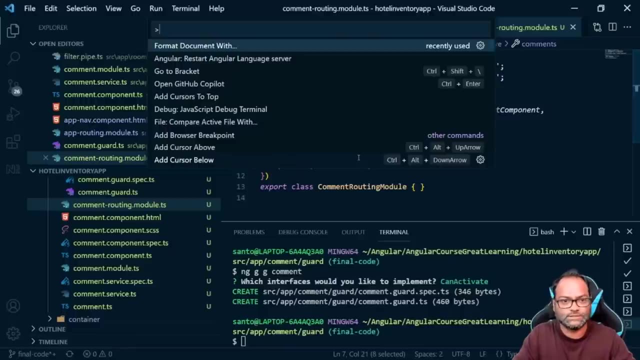 is a key value pair, so you can say comments, this is the key, and then you can say, okay, this is the comment resolver. why is this not available comments coming back? okay, great, so now this will be returning the comments data and let's see how we can actually access this. 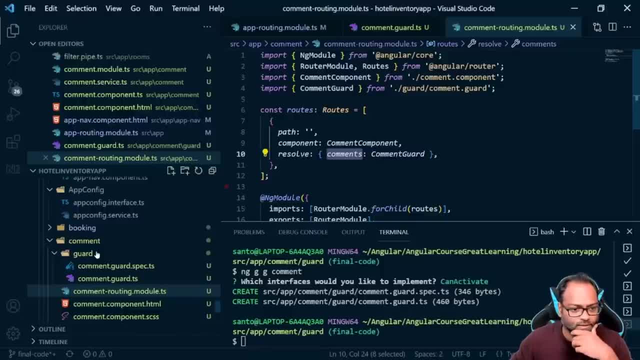 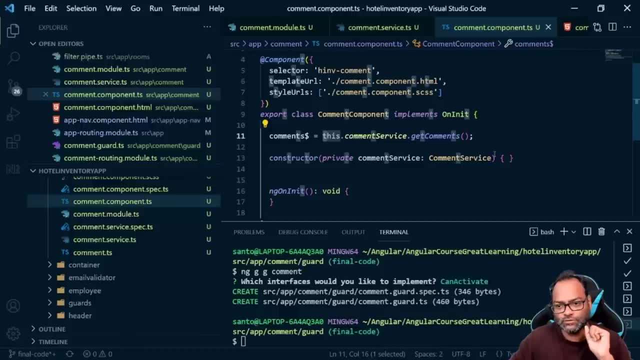 so this is the key, remember this. and to access this data. now we can go to component and here let's use what. do you think which service will be used here? remember when we talked spoke about router, we spoke about a service called activated route, we said anything related to data. 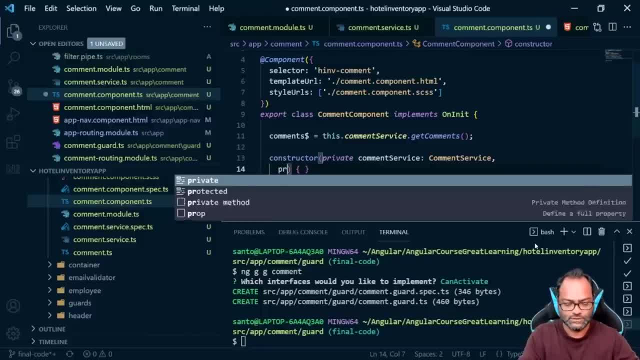 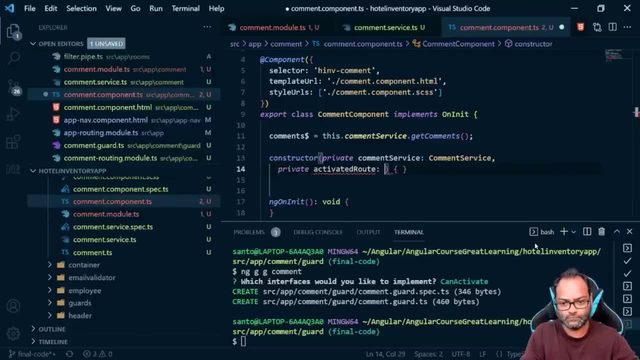 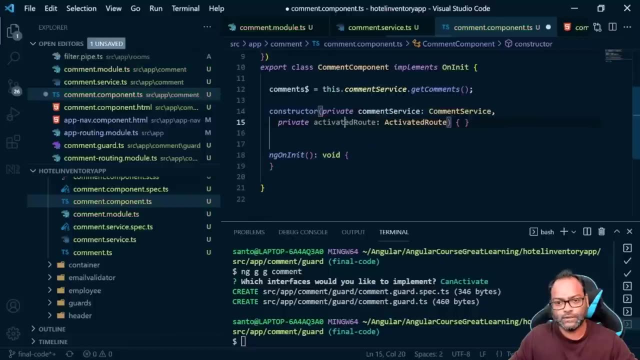 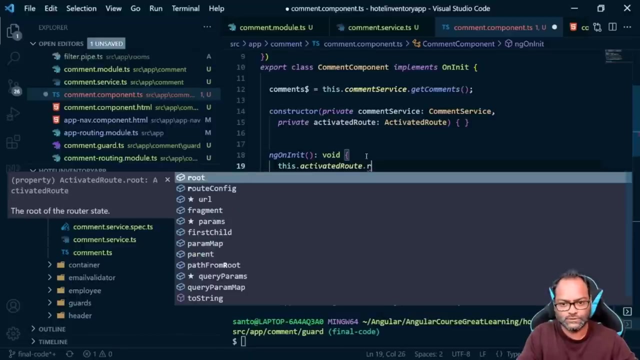 you should use the activated route service. so here we will of course use the same and first try to see if this data is available. so we'll what we'll do is activated route dot. so we'll say data dot, subscribe, and let's see what we get here. 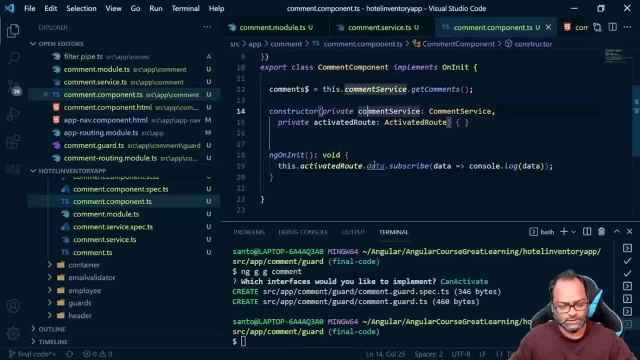 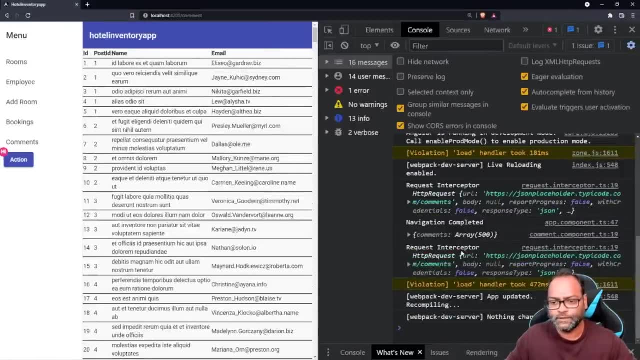 and we comment this out. or let's let let it be as of now, let's see, and we comment this out, or let's let let it be as of now, let's see, and we can see this comment. component dot t is line number 19, which is actually giving us. 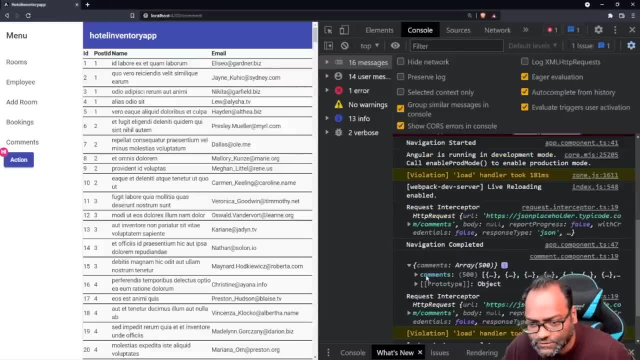 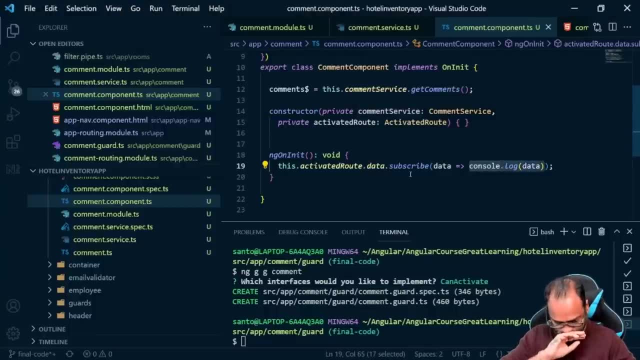 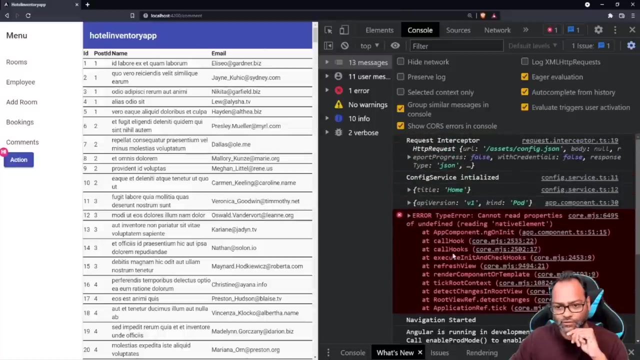 sorry- which is also giving us this key. so you can see it has a key- comments- and then it has 500 records. so let's try to access data dot. we can do something like this and let's see. so now we will get the 500 records rather than that which. 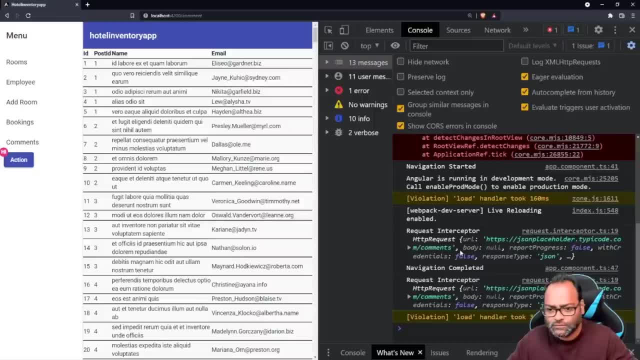 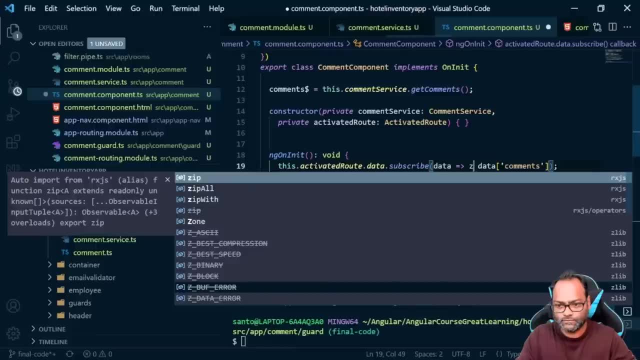 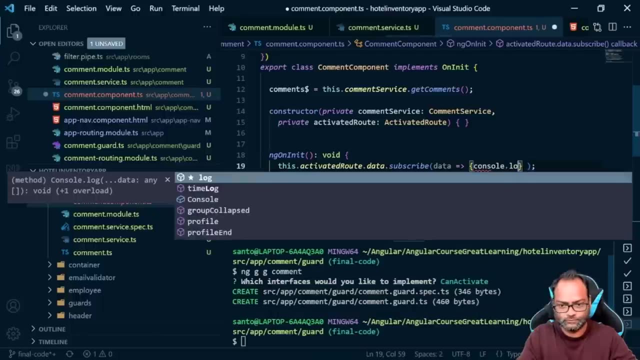 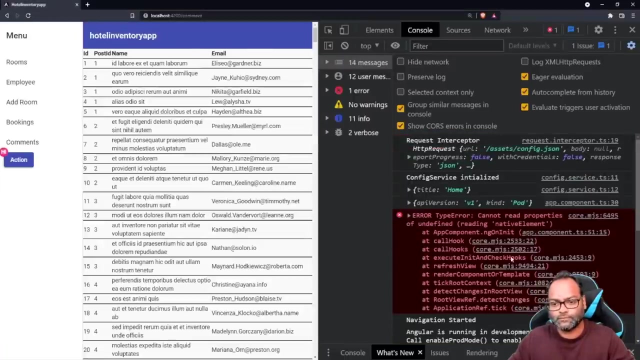 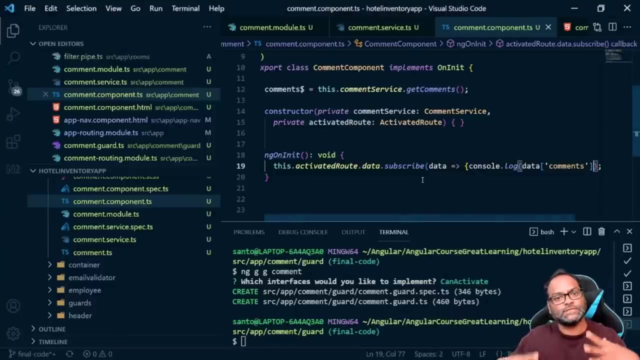 i'll just miss the consolelog and let's see if you can see that here and here it is. so we have all the 500 records available and we have this data prefaced. it's not like we are actually navigating to the route and then getting the data. no, we are pre-fetching the data. 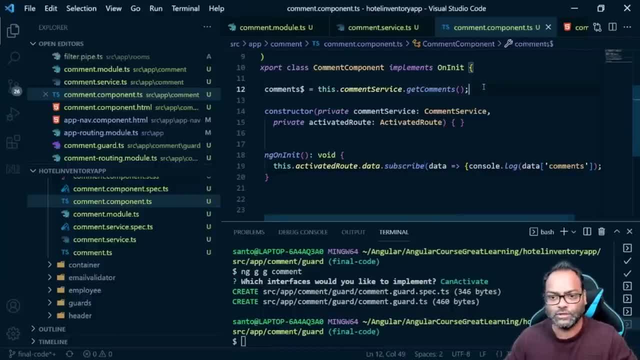 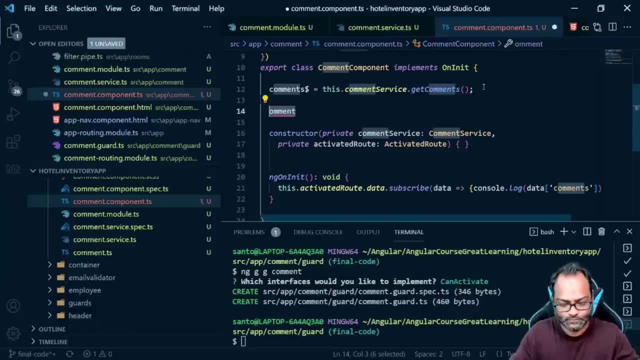 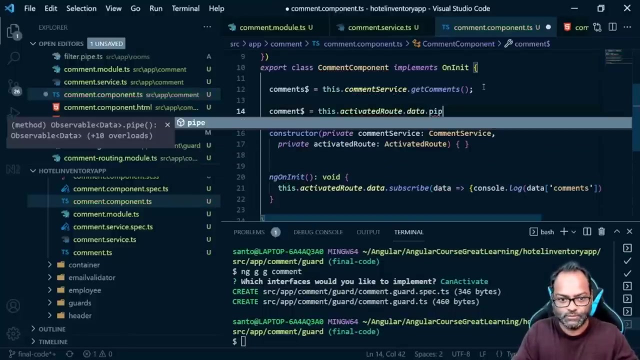 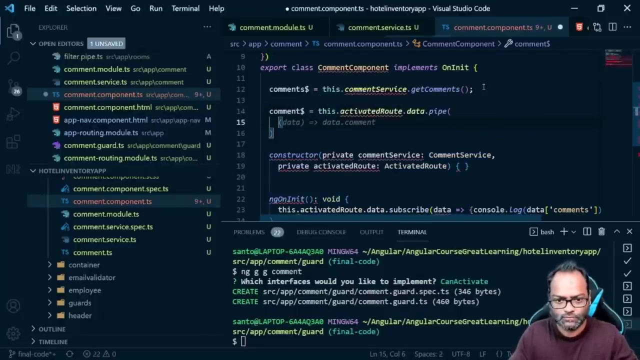 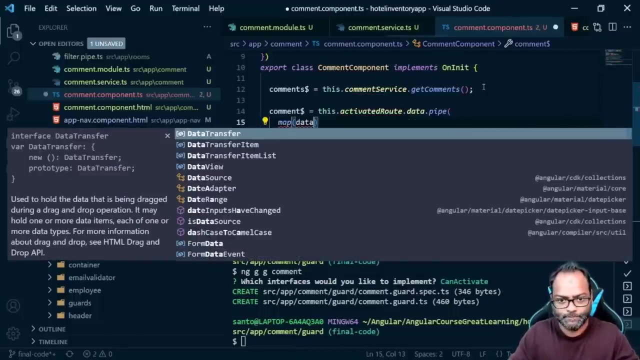 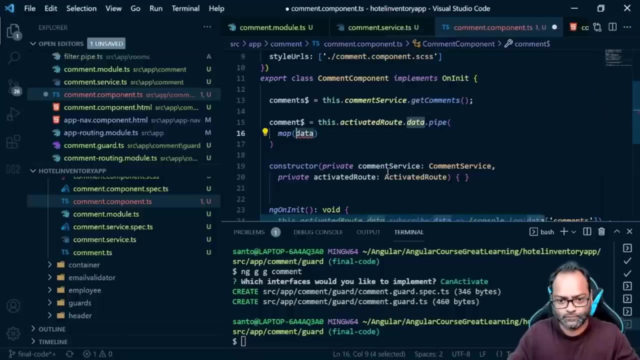 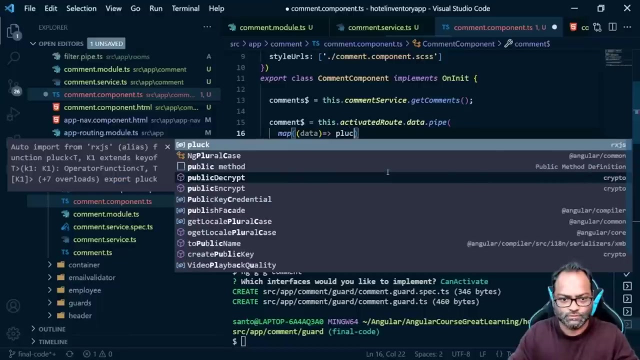 here we can also do something like this. let's try to use it as a stream so I can say this: comments string is this: dot activated route, dot data, and then we can use pipe of data, and here we can do pipe map data and we can use pluck to get the comments. let's see, let's try this. 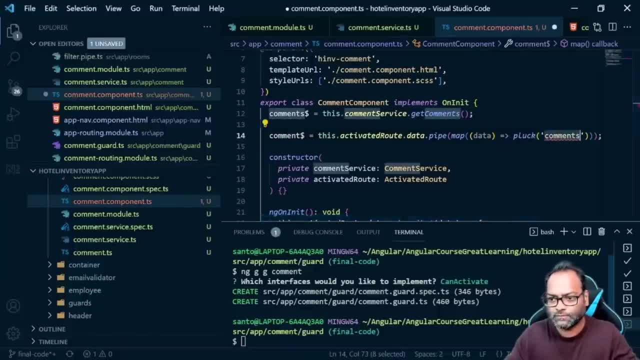 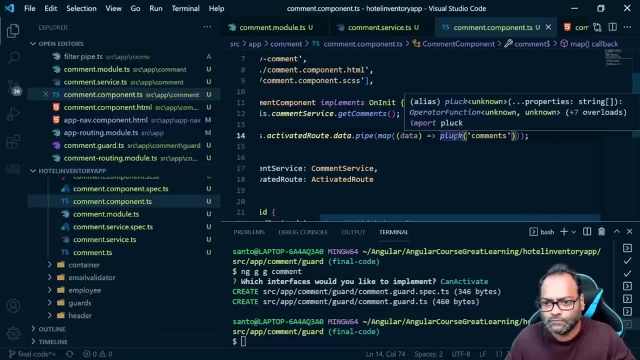 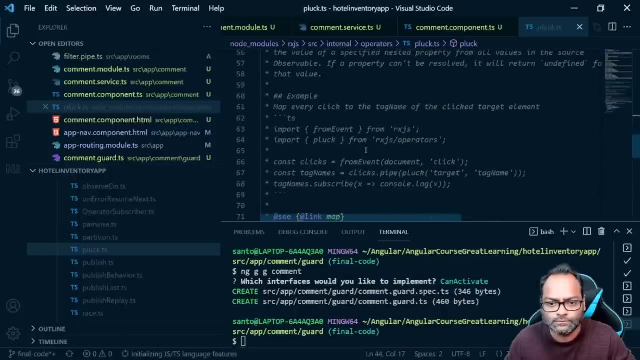 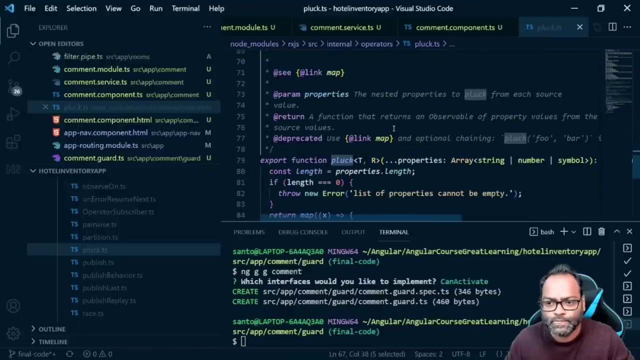 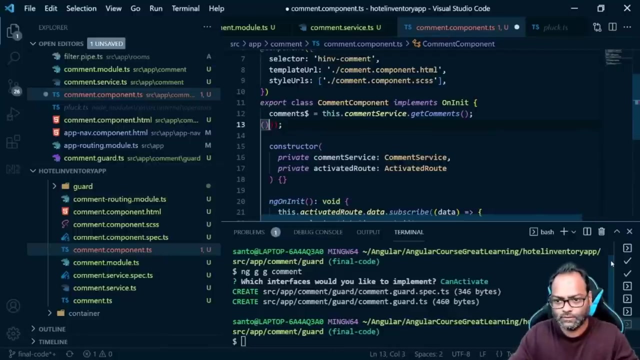 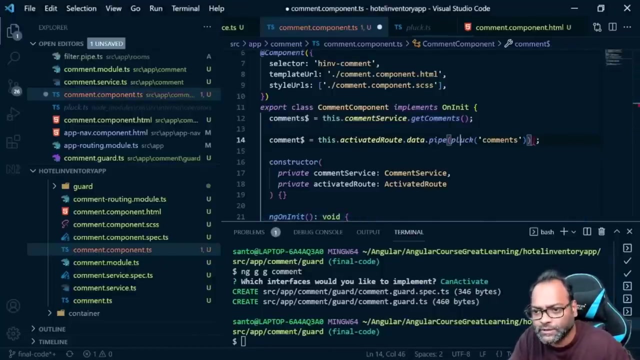 out see if this is the correct use case. okay, no, we can apply. look here. sorry, this is not the way to use it. so we can just use this pluck operator here and then we can define what key want. we want to access. this is it? so we can say, okay, this. 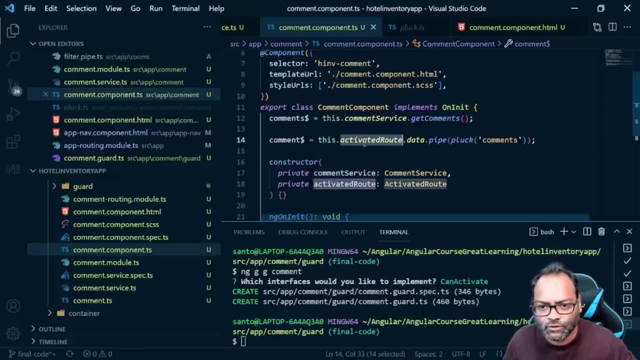 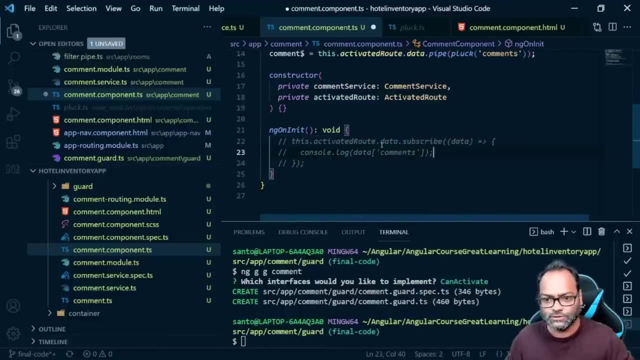 comment is: we are getting this comment from activated route data dot pipe and then we are plucking this particular key from the stream and we can remove this. now we don't need it. I was just writing it to show you, in case you want to subscribe, how you can do, how you can actually do that. let's. 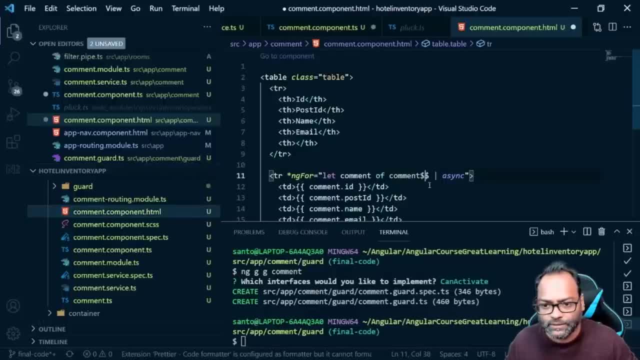 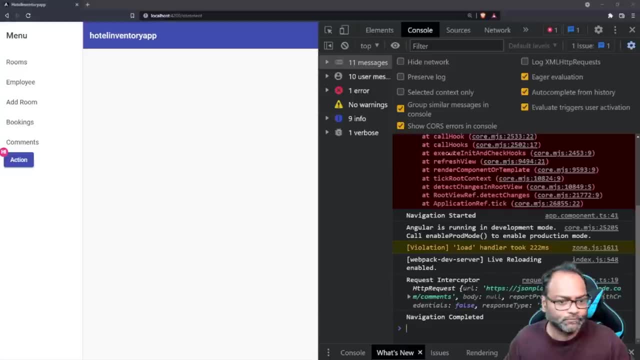 see the stream now. so rather than comments, I'll be using comment and see if it works. so let's save this and save this. okay, now let's go ahead and move from comments- sorry, move from any other route to comments. you can see that it's working, so let's go ahead. 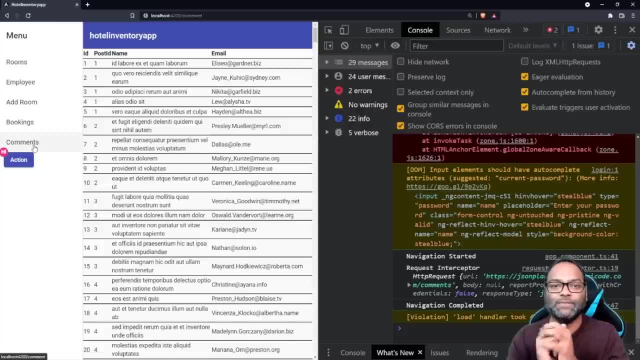 can actually across to the jungler here, and we can see that all of the two paths are then to search the data jelly language. so what we want to do here is actually say that this is the data we need to save and if you and Sikhy, can you go ahead. 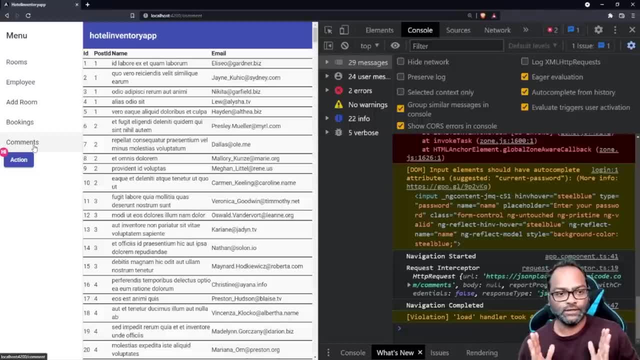 and first we're going to use for anything, and let's first go ahead and search the one path again. the, this kind of involves really an 10-24-15 field next to this field and all we have to do are, instead of the data generally, we have to restrict it, because so this relevance 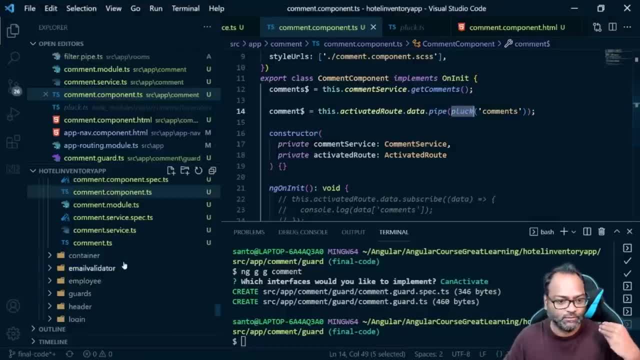 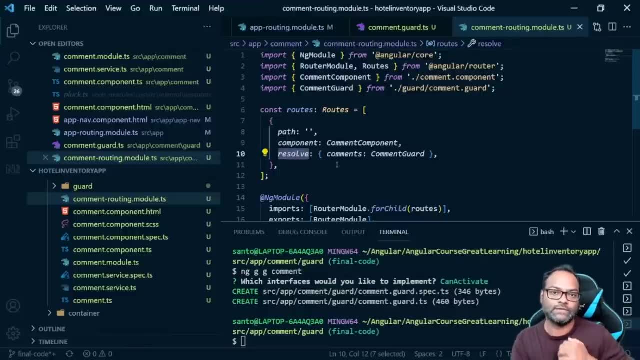 is just it's not going to work. depends have to be there. cup button for that answer in terms ofoe it into your route. so we already added this into our resolve card. so we are saying, okay, before you migrate, or sorry, before you navigate to this route, go ahead and pre-fetch this data. 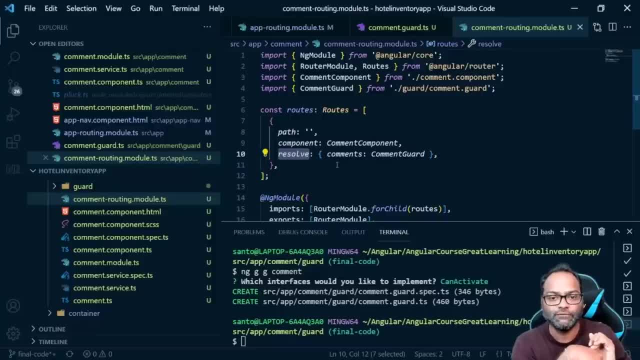 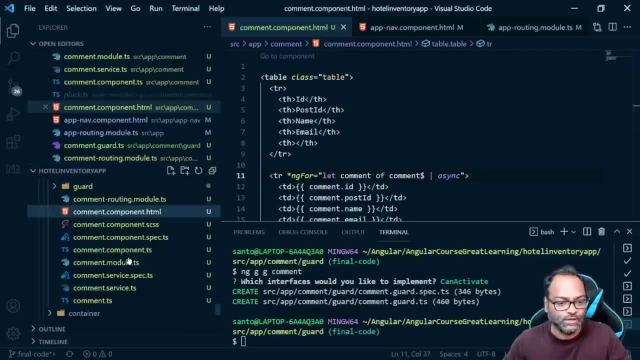 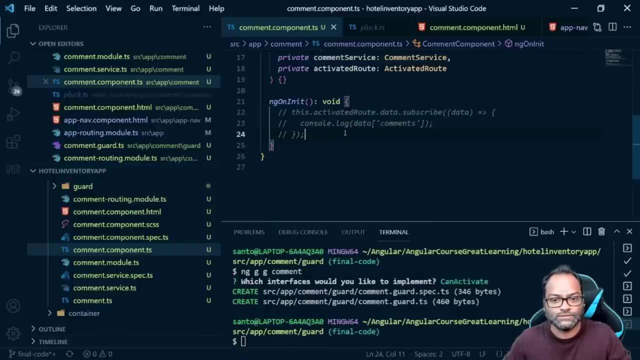 so this data should be available before my user will navigate to this. so this is another use case for using the pre-fetch- or you can say resolve- card. so i am keeping the same both the ways. feel free to use whatever fits your scenario. i have also this code available in case you don't. 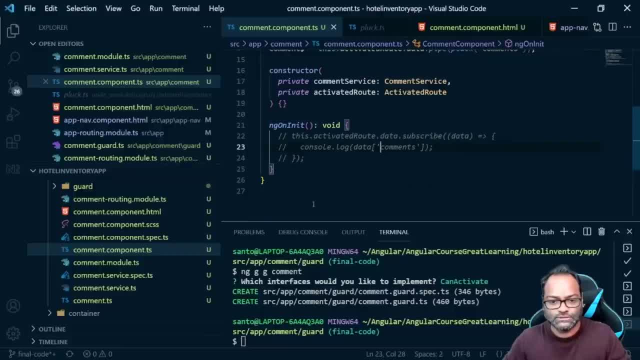 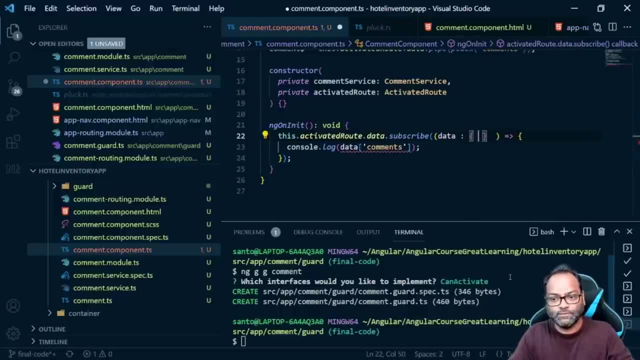 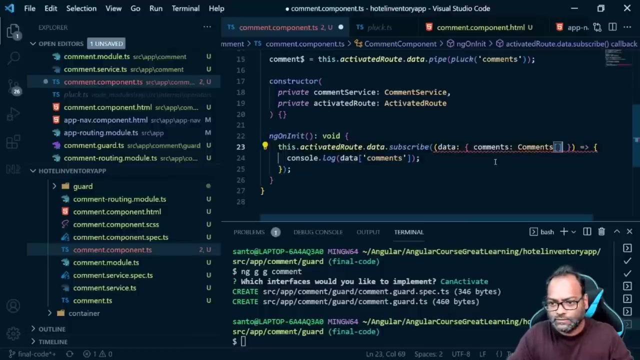 think that there's something which you need. generally, we should not use this. let me show you a better way to do this. you can actually do something like this. you can provide the type, so you can say: okay, this is, this will be my comment. you comments which will be type of comments array, so then this should work. 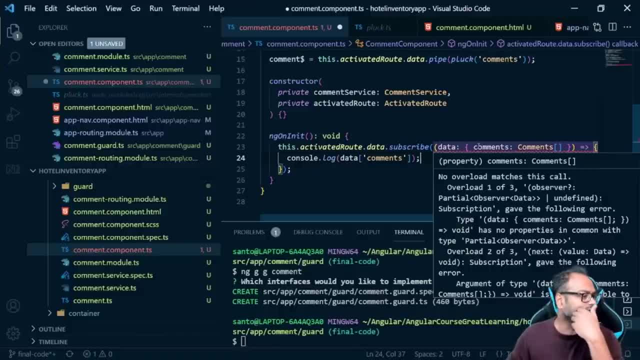 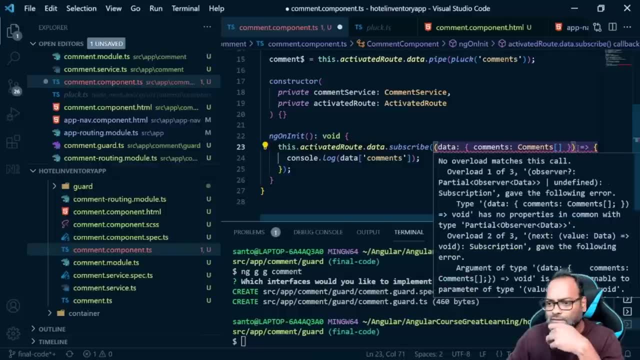 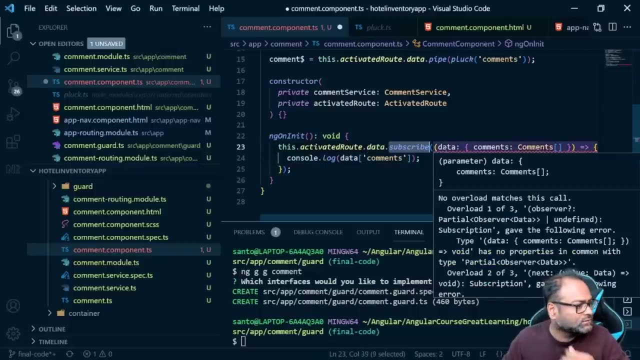 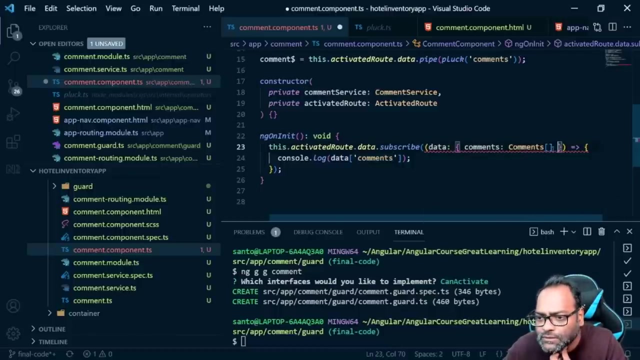 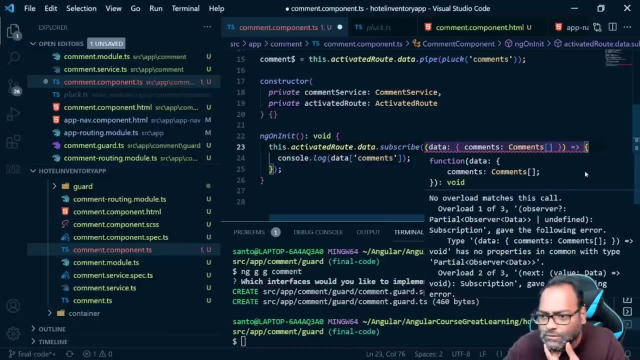 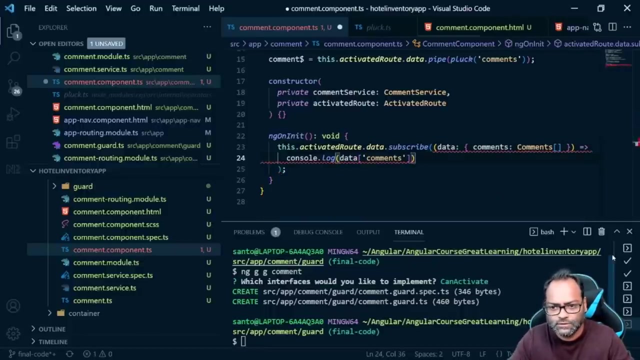 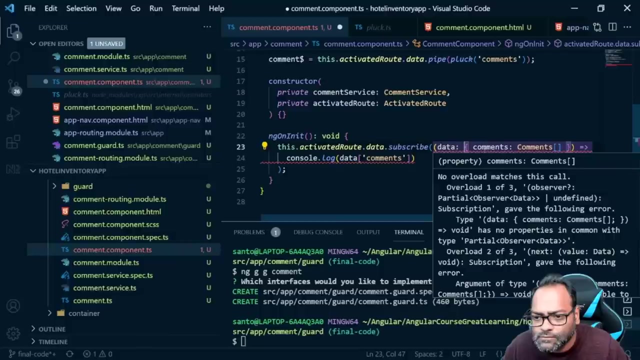 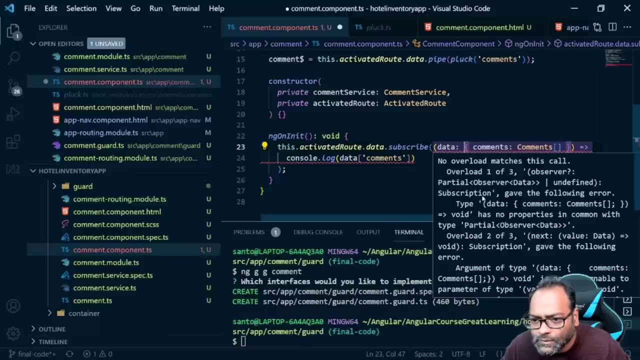 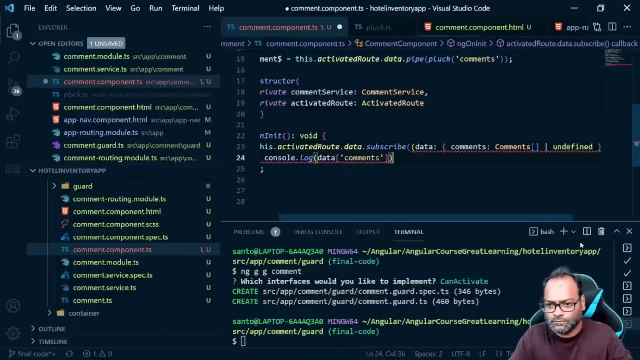 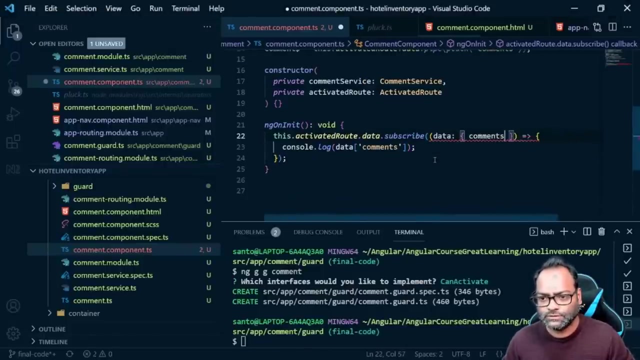 no load matches this call, so create anonymous function. comments and comments is type of this array. let's see it works. no, somehow strange. this is the best way we can do this. let me just remove it so we can say data and here, uh, you can typecast. here, so you. 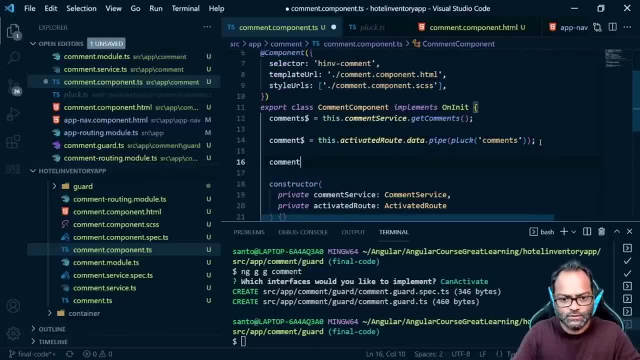 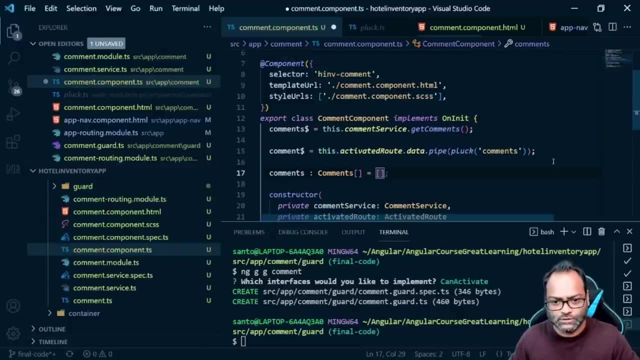 here, uh, you can typecast here, so you here, uh, you can typecast here, so you can actually create a common creator, can actually create a common creator, can actually create a common creator: property, property, property, comments, which is type of comments, comments, comments array, array, array is equals to this, and then you can say: 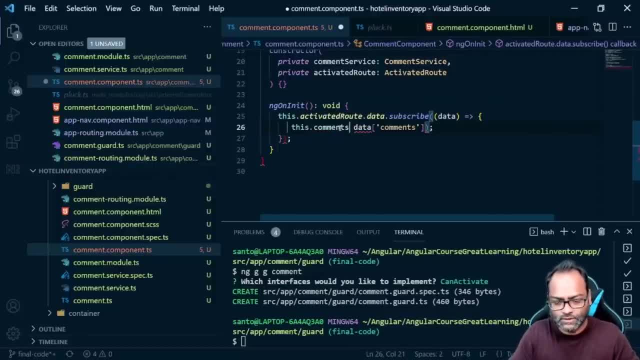 is equals to this, and then you can say: is equals to this, and then you can say that this dot, that this dot, that this dot comments, comments, comments- is equals to data of type this. so this is: is equals to data of type this. so this is: is equals to data of type this. so this is how you can uh do it. 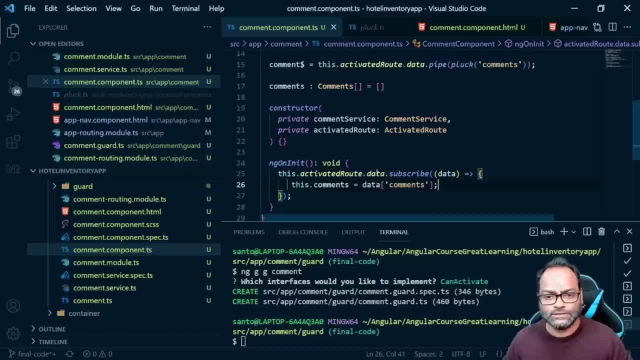 how you can uh do it, how you can uh do it, and you will get the typing after this, and you will get the typing after this, and you will get the typing after this. so, uh, in case, these are three ways. so, uh, in case, these are three ways. 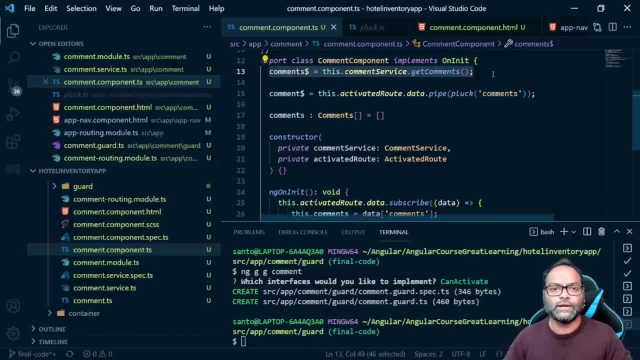 so, uh, in case, these are three ways. here we call the method to get the data. here we call the method to get the data. here we call the method to get the data after we landed on the view. this is after we landed on the view. this is: 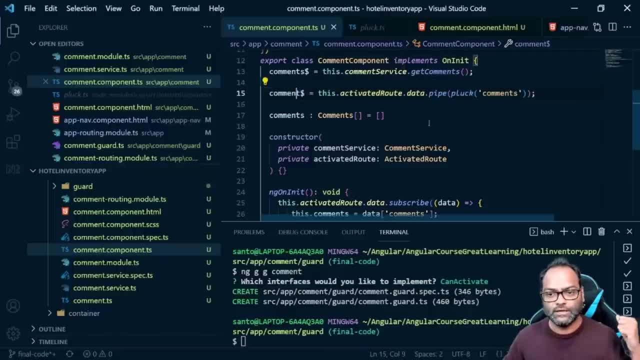 after we landed on the view. this is using the resolve method and we use the using the resolve method and we use the using the resolve method and we use the stream we uh. we have not used uh the stream we uh. we have not used uh the stream we uh. we have not used uh the subscribe method. we have not manually. 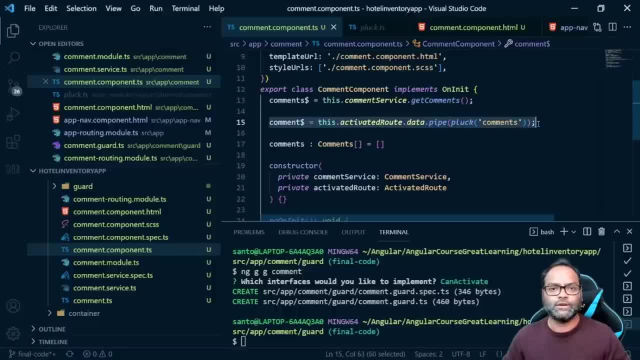 subscribe method. we have not manually subscribe method. we have not manually subscribed which we did here, subscribed which we did here, subscribed which we did here. but uh, choose one which fits your. but uh, choose one which fits your, but uh, choose one which fits your scenario. now, in this video, we are going to talk. 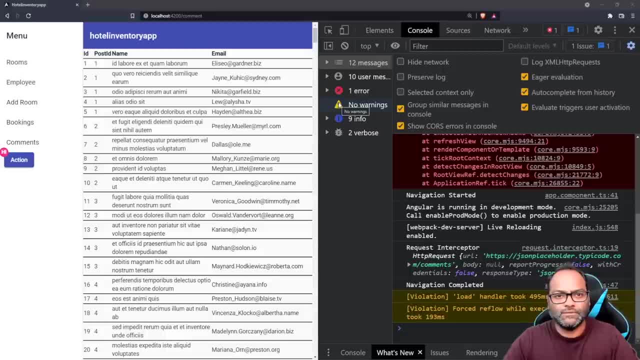 now in this video we are going to talk. now in this video we are going to talk about how you can do global error, about how you can do global error, about how you can do global error handling. we have seen, like uh, how we can handling. we have seen, like uh, how we can. 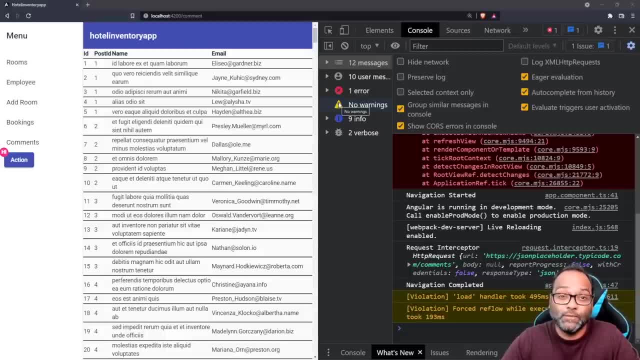 handling. we have seen like: uh, how we can do error handling for http service, but do error handling for http service, but do error handling for http service. but what in case we want to do it at global? what in case we want to do it at global? what in case we want to do it at global level? 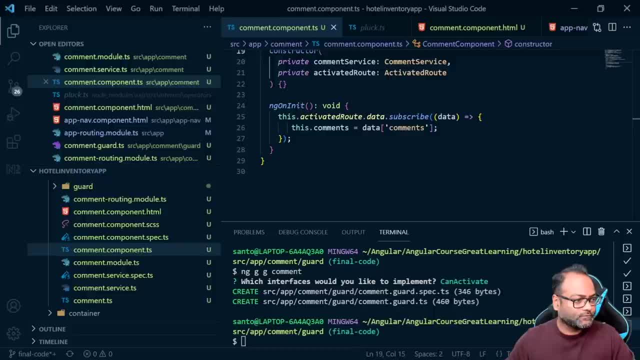 level level. okay, so let's go ahead and try that out. okay, so, let's go ahead and try that out. okay, so let's go ahead and try that out. so angular provides you a, so angular provides you a, so angular provides you a class, class, class, that's a class. 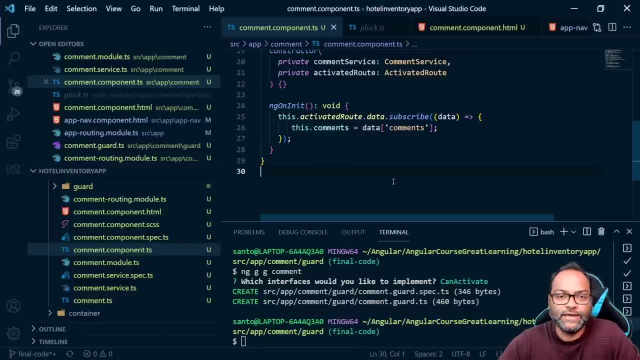 that's a class. that's a class, so angle provides you a service which so angle. provides you a service which so angle provides you a service which is already available, called error, and is already available called error, and is already available called error and handler. so handler, so. 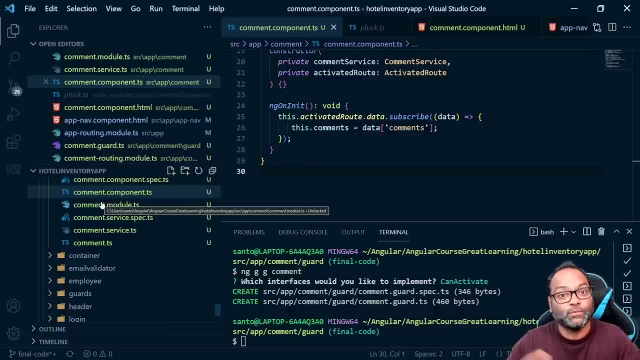 handler. so what you can do is you can actually extend. what you can do is you can actually extend. what you can do is you can actually extend that particular service and you can that particular service and you can that particular service and you can provide your own info. 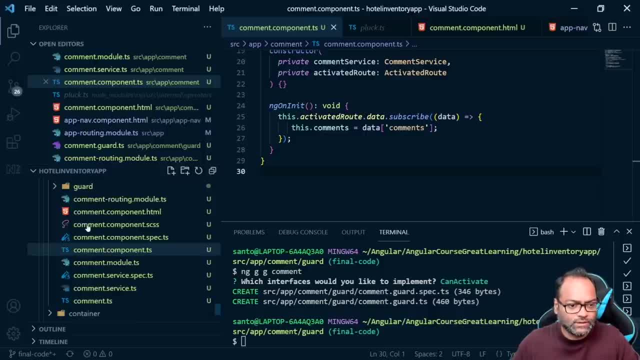 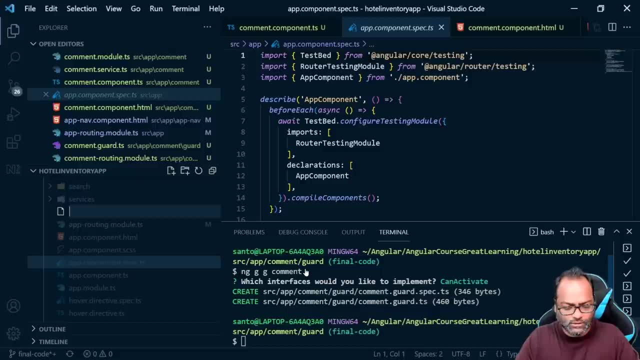 provide your own info, provide your own info, your own implementation, your own implementation, your own implementation. so here let's uh, so here let's uh, so here let's uh. go ahead and do that, so i'll create a class, so i'll create a class. so i'll create a class here called 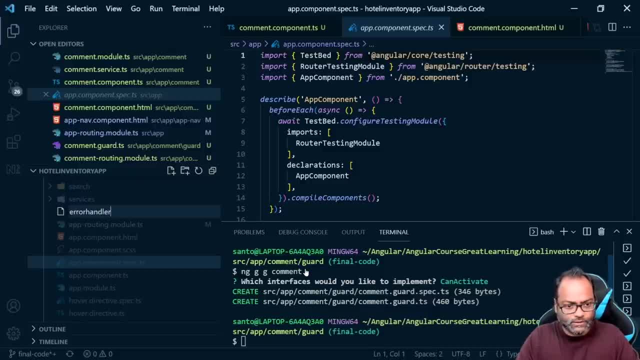 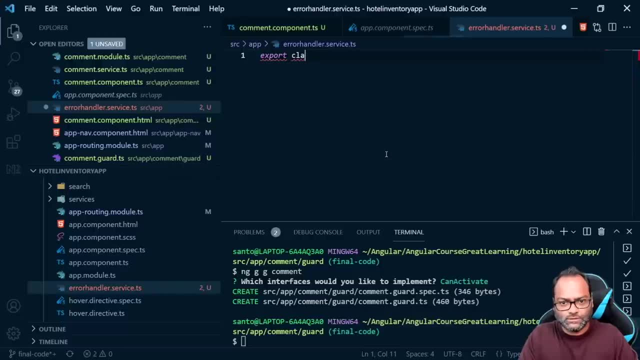 here called, here called error handler handler handler surface surface surface dot ds, dot ds, dot ds. and we'll create this class export class and we'll create this class export class and we'll create this class export class and we'll call it as: and we'll call it as: 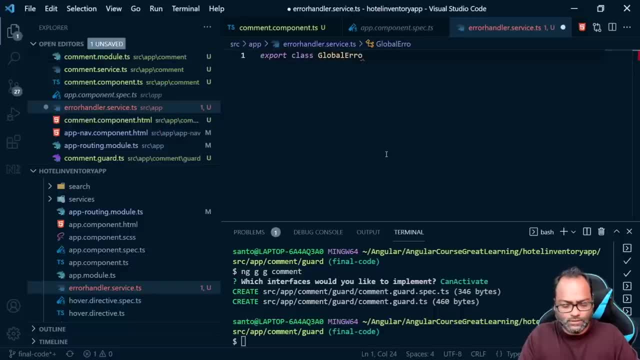 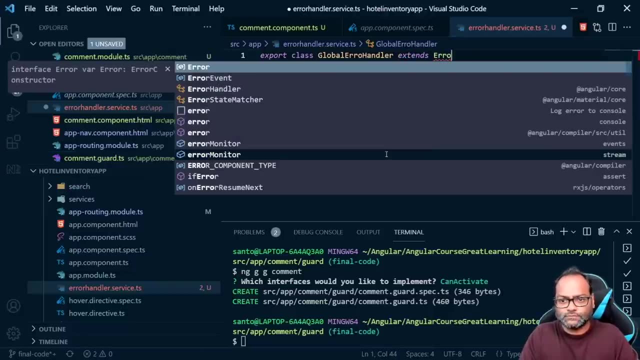 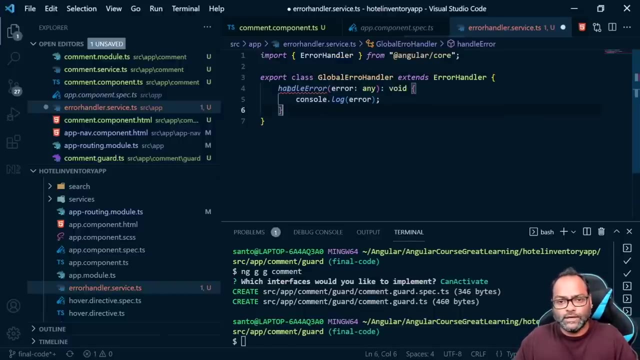 and we'll call it as global, global, global error, error, error handler, handler, handler which extends, which extends, which extends error handler. and now, uh, you can just call the handle, and now, uh, you can just call the handle, and now, uh, you can just call the handle error method. 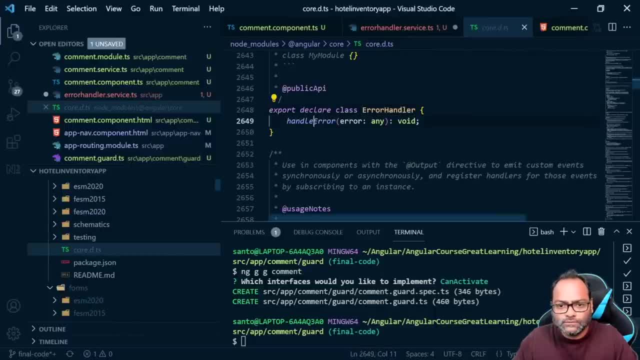 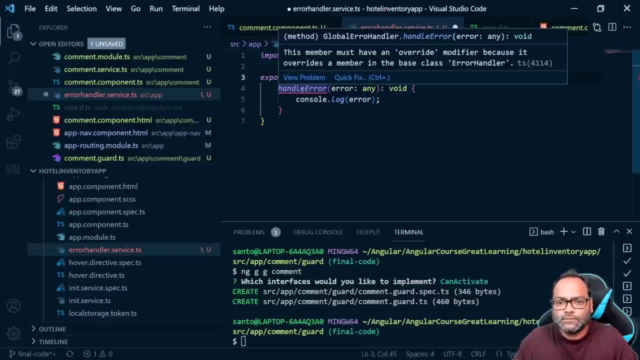 error method: error method. so, let's see, so, let's see, so, let's see, this must have an overrate. okay, let's see, so we have uh error. okay, let's see, so we have uh error. okay, let's see, so we have uh error. handler handler. 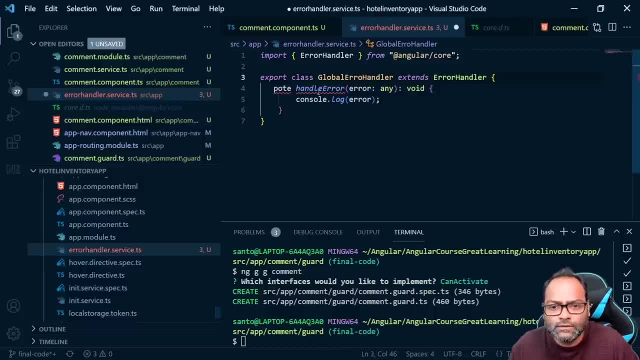 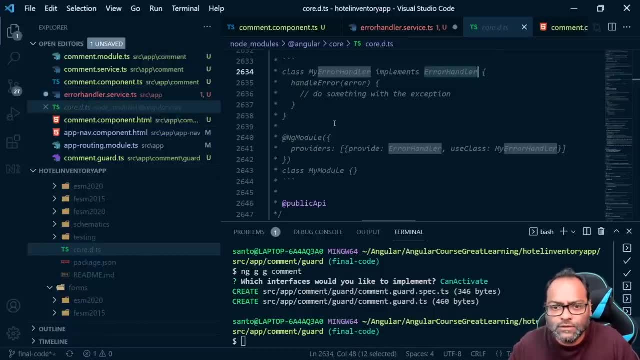 handler. uh implements error handler and uh implements error handler. and uh implements error handler and handle error which does something. so i'm handle error which does something. so i'm handle error which does something. so i'm just wondering what's just wondering? what's just wondering what's wrong here? that should be. 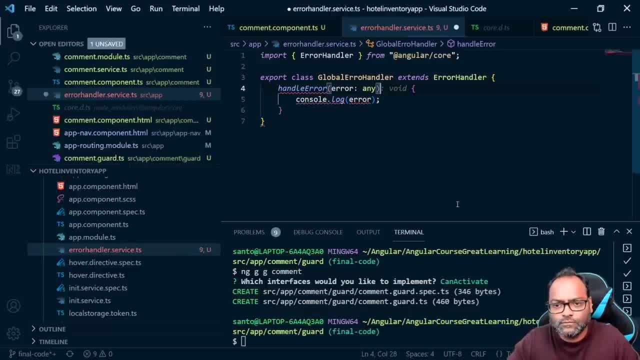 wrong here. that should be wrong here. that should be okay. you okay, you okay. you looks correct to me, okay, sorry. implements looks correct to me, okay, sorry. implements looks correct to me, okay, sorry. implements implements error handler, and then uh, it's. implements error handler, and then uh, it's. implements error handler. and then, uh, it's, it's a. actually, you can see, it's a. it's a. actually, you can see it's a class, but you can also implement it. it's a, actually, you can see, it's a class, but you can also implement it. 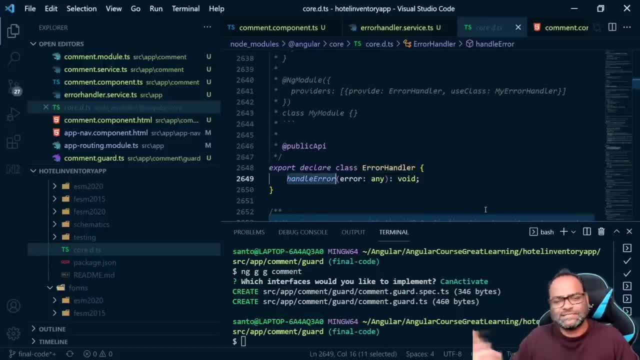 it's a, actually you can see, it's a class, but you can also implement it because it provides a single, because it provides a single, because it provides a single method which is method, which is method, which is just like a method definition, not just like a method definition, not. 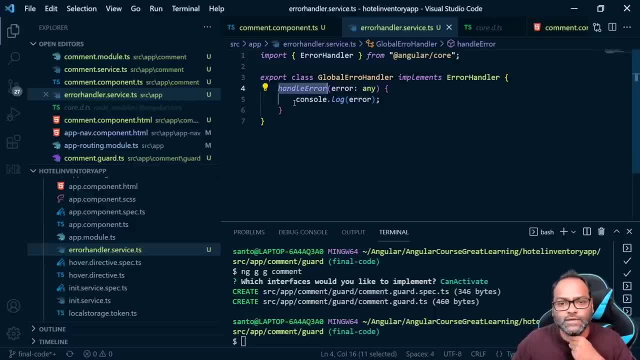 just like a method definition, not implementation. so i can just go ahead and implementation. so i can just go ahead and implementation, so i can just go ahead and implement it, and then we are just doing implement it, and then we are just doing implement it, and then we are just doing consolelog right now. 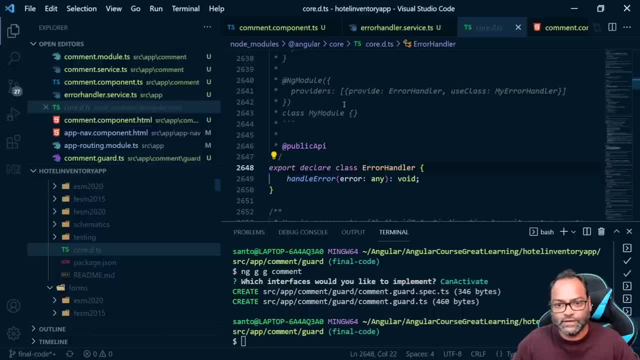 consolelog right now. consolelog right now. now to handle this, to register this. you now to handle this to register this. you now to handle this, to register this. you can, of course, go ahead and see how we can, of course, go ahead and see how we can, of course, go ahead and see how we can do it. so you have to go ahead and add. 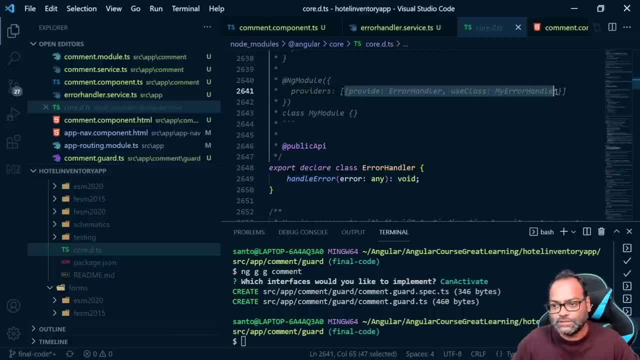 can do it, so you have to go ahead and add. can do it, so you have to go ahead and add it into providers, it into providers, it into providers, like this. so let's copy this like this, so let's copy this like this. so let's copy this and let's go to our app module, because 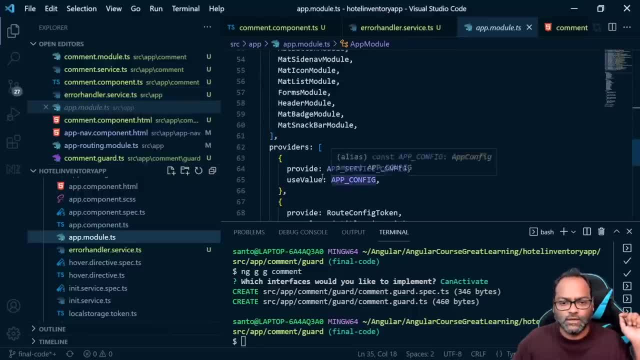 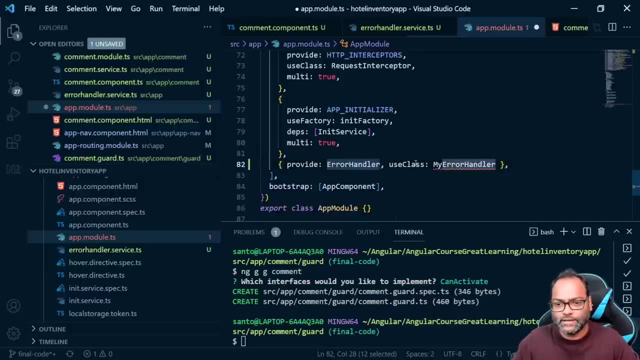 and let's go to our app module because- and let's go to our app module because we want to actually handle the, we want to actually handle the, we want to actually handle the error at global level, and we'll say, okay, this is provide error. and we'll say, okay, this is provide error. 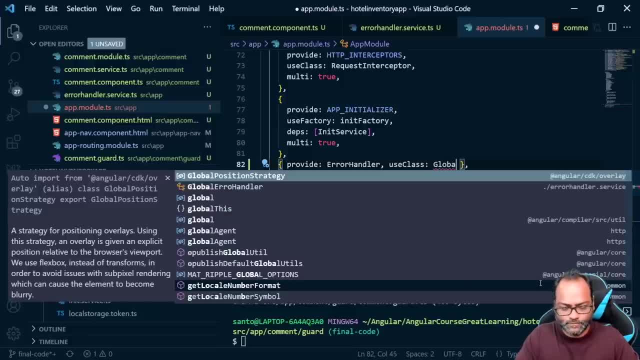 and we'll say, okay, this is provide error handler, and then handler, and then handler, and then this is our global error handler plus. this is our global error handler plus. this is our global error handler plus. now we need to introduce some error. now we need to introduce some error. 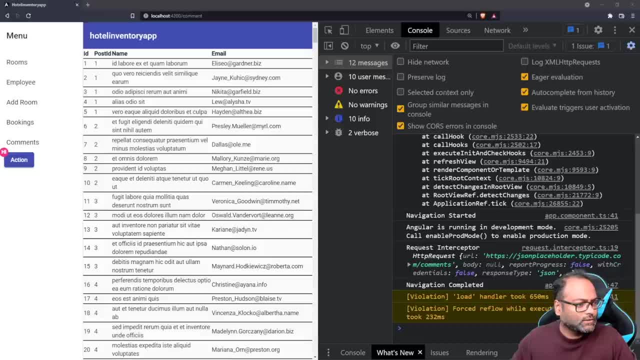 now we need to introduce some error. let's do that. let's verify if it is working fine, right, let's verify if it is working fine, right, let's verify if it is working fine right now. so now, so now. so okay, nothing, uh, no issue. so what we will? 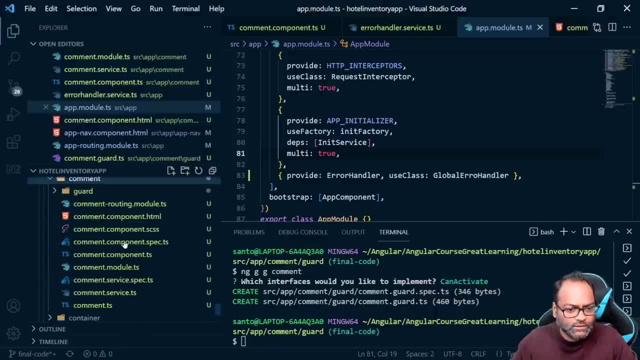 okay, nothing, uh, no issue. so what? we will? okay, nothing, uh, no issue. so what we will do is: we will go to this, do is. we will go to this, do is. we will go to this comment, api comment, api comment, api, comment service. and then we will just 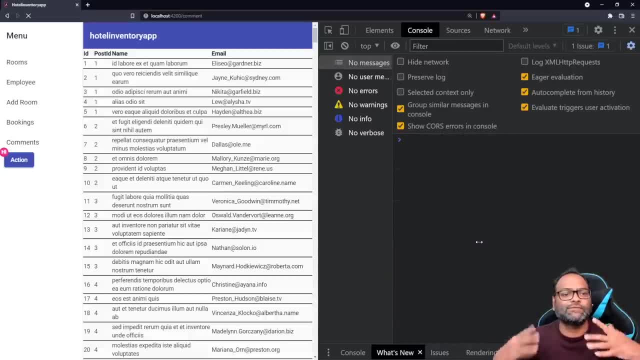 comment service, and then we will just comment service, and then we will just make some mistake here, right so this make some mistake here, right so this make some mistake here, right so this api does not exist and it will throw an. api does not exist and it will throw an. 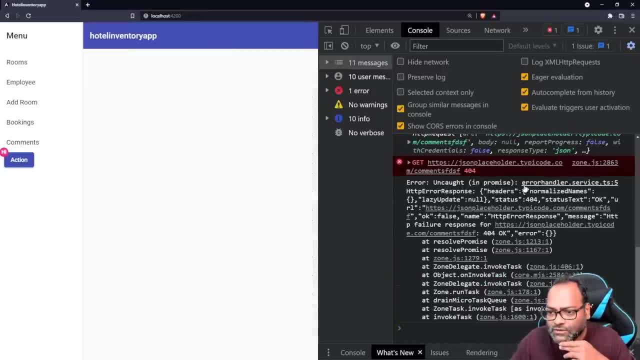 api does not exist and it will throw an exception, exception. exception. now you can see. uh, there is an error. now you can see. uh, there is an error. now you can see. uh, there is an error. handler line number. handler line number. handler line number five, which says http error response and. 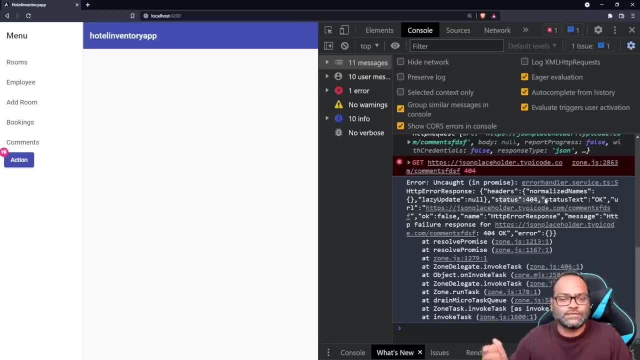 five which says http error response, and five which says http error response. and this says okay, this api does not exist. this says okay, this api does not exist. this says okay, this api does not exist. right, or the status code is 404, it means right, or the status code is 404- it means. 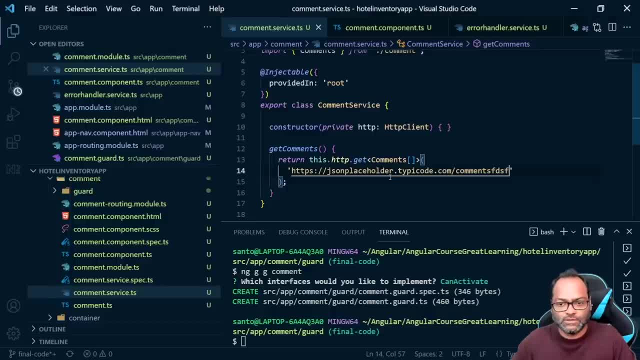 right or the status code is 404. it means it is not able to. it is not able to. it is not able to go ahead and catch this particular api or go ahead and catch this particular api. or go ahead and catch this particular api or go ahead and access this particular api. 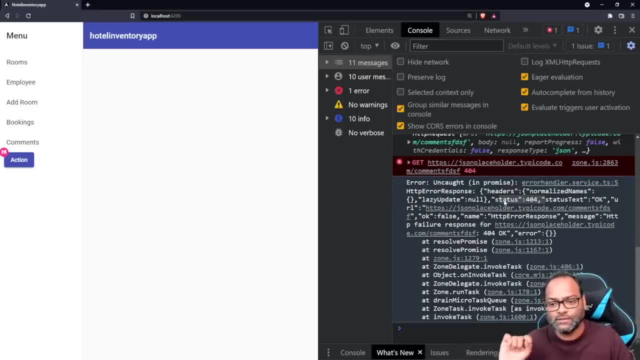 go ahead and access this particular api. go ahead and access this particular api. so it says, okay, it does not exist. so it says, okay, it does not exist. so it says, okay, it does not exist. and we are able to handle this exception. and we are able to handle this exception. 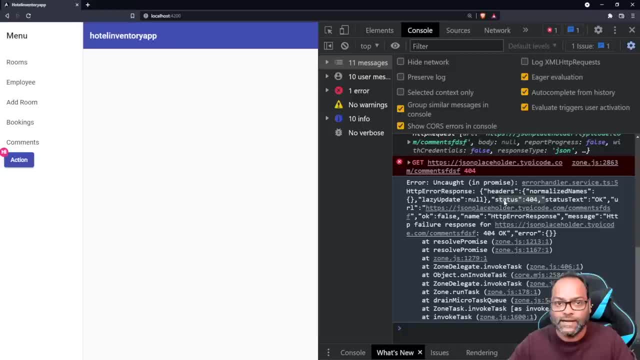 and we are able to handle this exception at global level by using our new global at global level, by using our new global at global level, by using our new global error handler class, error handler class, error handler class, and, and you can do uh more right, i mean, it's not uh. 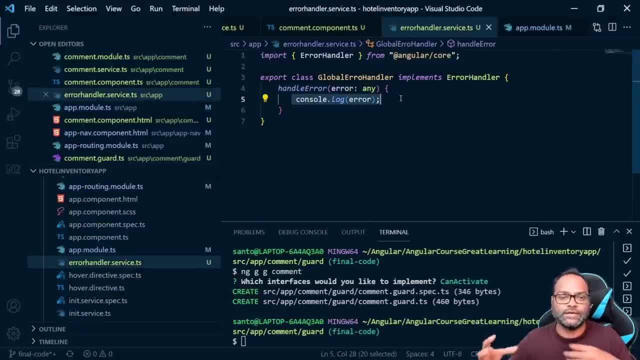 you can do uh more, right, i mean, it's not uh. you can do uh more, right, i mean it's not uh. in our example, we are just using the. in our example, we are just using the. in our example, we are just using the consolelog, but you can actually send it. 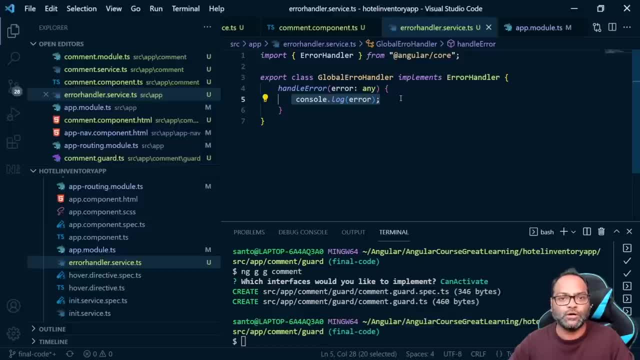 consolelog, but you can actually send it consolelog. but you can actually send it to your, to your, to your backend, or you can actually send it to backend, or you can actually send it to backend, or you can actually send it to your. whatever apis which you have. 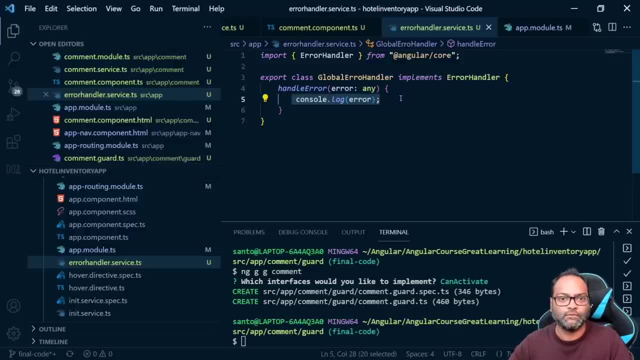 your whatever apis which you have, your whatever apis which you have, and you can save this error somewhere and you can save this error somewhere and you can save this error somewhere. so, whenever you are revisiting your like, so whenever you are revisiting your like, so whenever you are revisiting your like error logs to see if there is some. 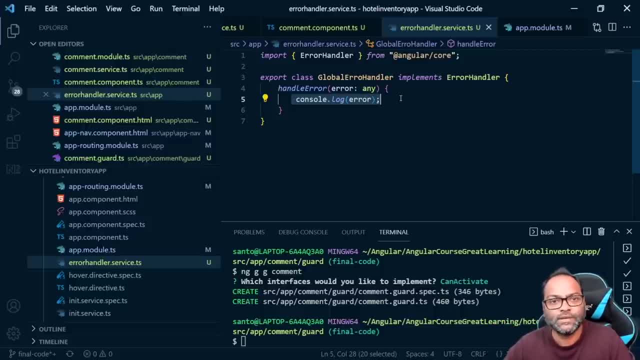 error logs to see if there is some error logs, to see if there is some problem, which problem, which problem which your users are facing? because there are, your users are facing because there are. your users are facing because there are some, some, some edge cases, right, we generally miss out. so 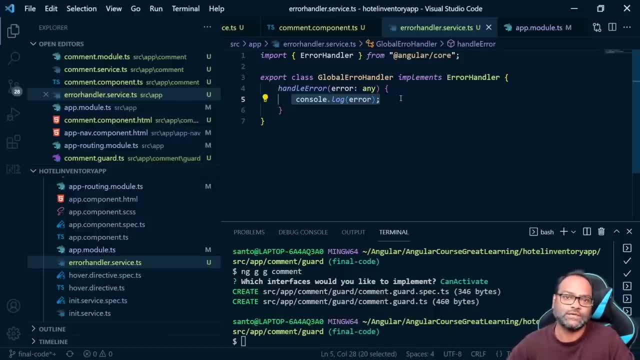 edge cases: right, we generally miss out. so edge cases- right, we generally miss out. so just go ahead and add error handler. just go ahead and add error handler. just go ahead and add error handler, class and class and class and log all the errors until unless your log all the errors, until unless your 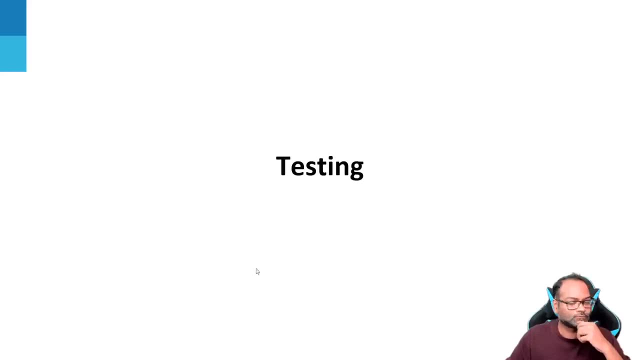 log all the errors until unless your application becomes stable, and then you application becomes stable, and then you application becomes stable and then you can remove it, can remove it, can remove it. let's talk a little bit about testing. let's talk a little bit about testing. let's talk a little bit about testing, of course, when, whenever you are working, 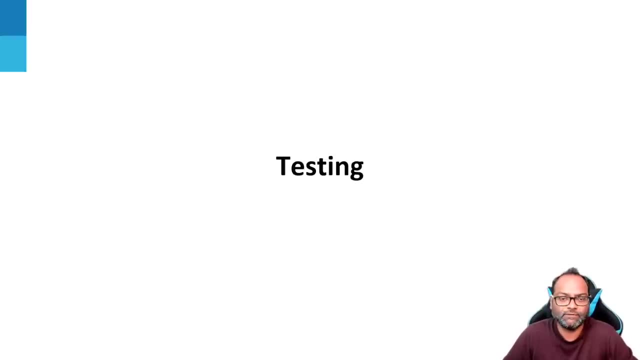 of course, when, whenever you are working, of course, when, whenever you are working on some application, you need to also on some application, you need to also on some application, you need to also write unit test cases. that's the write unit test cases. that's the write unit test cases. that's the developer's job. 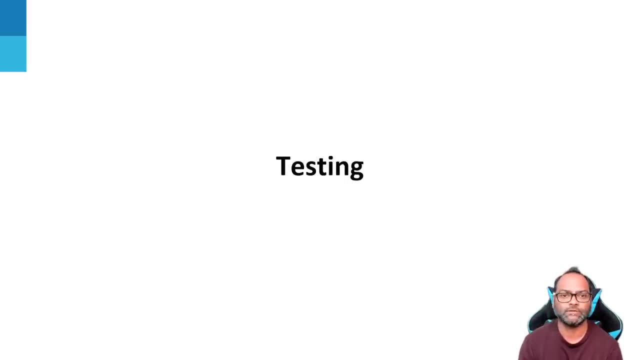 developer's job, developer's job. but there are many types of testing which. but there are many types of testing which. but there are many types of testing which is uh, is uh, is uh, which is done. so we have unit test cases. which is done, so we have unit test cases. 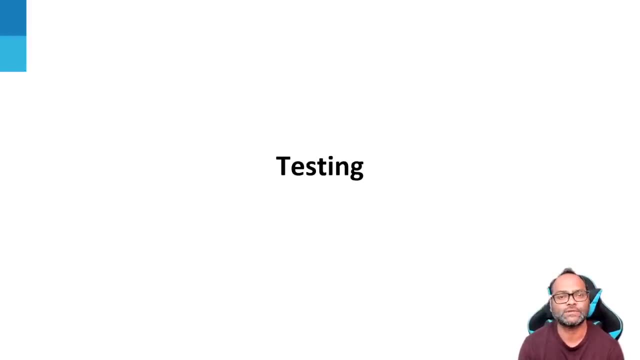 which is done. so we have unit test cases, or unit testing which is written by, or unit testing which is written by, or unit testing which is written by developers, and then you also have developers, and then you also have developers, and then you also have something known as integration test, or 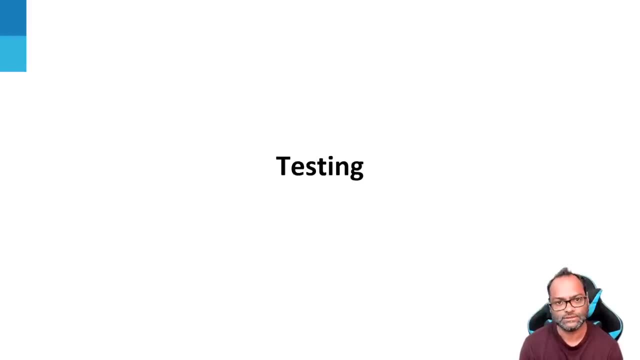 something known as integration test, or something known as integration test, or end-to-end test, which is generally done, end-to-end test, which is generally done, end-to-end test, which is generally done by the testers, so by the testers, so by the testers. so the tools are a little bit different. so 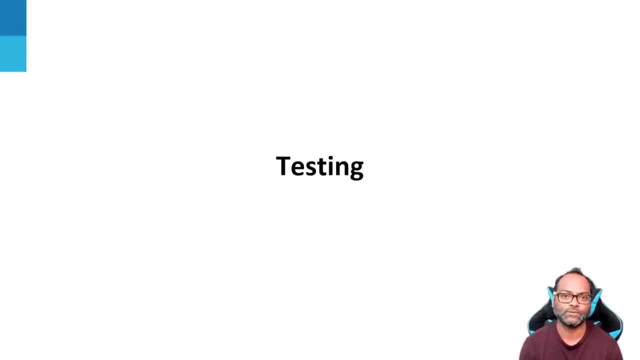 the tools are a little bit different, so the tools are a little bit different. so, for example, for end-to-end testing, for example for end-to-end testing, for example for end-to-end testing tests, you can use something known as tests. you can use something known as. 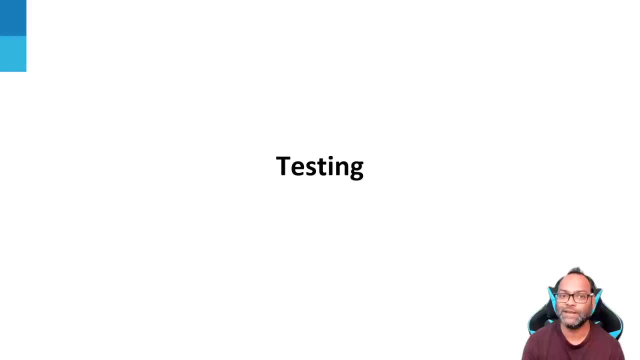 tests. you can use something known as cypress, cypress, cypress, or there are other tools like playwright, or there are other tools like playwright, or there are other tools like playwright, which is also available. you can use, which is also available. you can use which is also available. you can use and a lot of older applications used to. 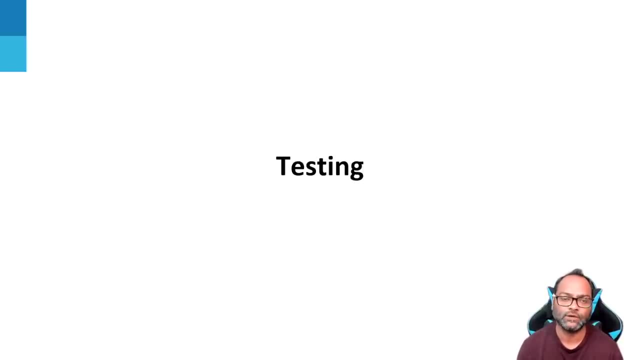 and a lot of older applications used to- and a lot of older applications used to have have have a protector, so protector is discontinued. a protector, so protector is discontinued. a protector, so protector is discontinued. now angular team decided to drop. now angular team decided to drop. now angular team decided to drop, maintaining it. so they are not. 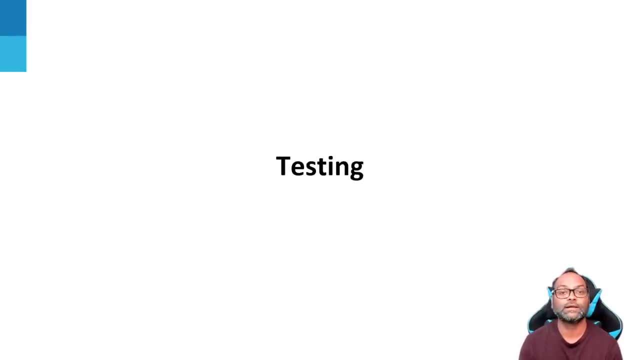 maintaining it, so they are not maintaining it, so they are not maintaining it anymore. and they have maintaining it anymore and they have maintaining it anymore. and they have also dropped this: dropped. creating an: also dropped- this dropped. creating an: also dropped- this dropped. creating an end-to-end application with 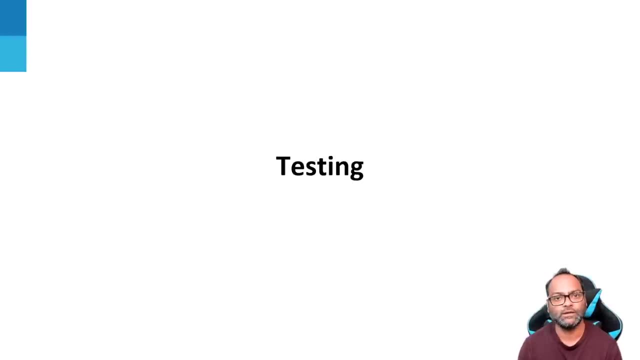 end-to-end application with end-to-end application with angular cli, so before angular cli, so before angular cli, so before before angular 12. they uh whenever used before angular 12. they uh whenever used angular 12. they uh whenever used to create a new application there used. 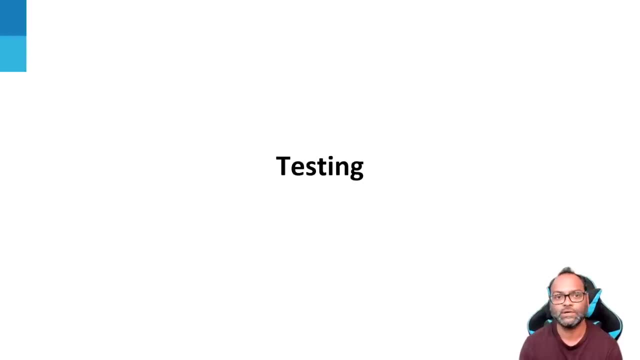 to create a new application there used to create a new application there used to be a end-to-end application as well, to be a end-to-end application as well, to be a end-to-end application as well. which used to be created, but now. which used to be created, but now. 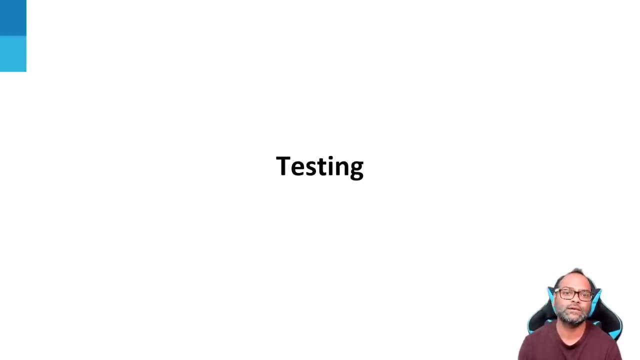 which used to be created, but now it is not created anymore, so you have. it is not created anymore, so you have, it is not created anymore. so you have to go ahead and add any, to go ahead and add any, to go ahead and add any compatible uh, end-to-end uh. 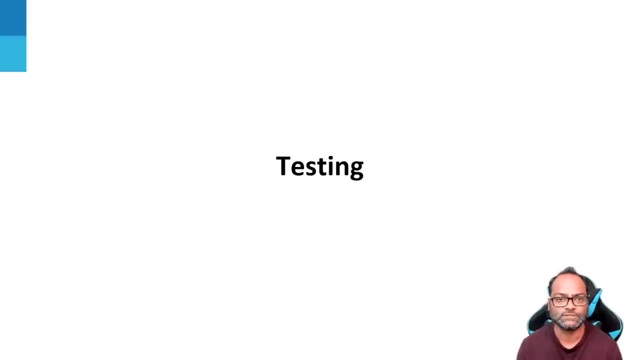 compatible uh end-to-end uh. compatible uh end-to-end uh. test suit to your application, so test suit to your application, so test suit to your application. so cypress is preferred, which is used by many. cypress is preferred, which is used by many. cypress is preferred, which is used by many large organizations. 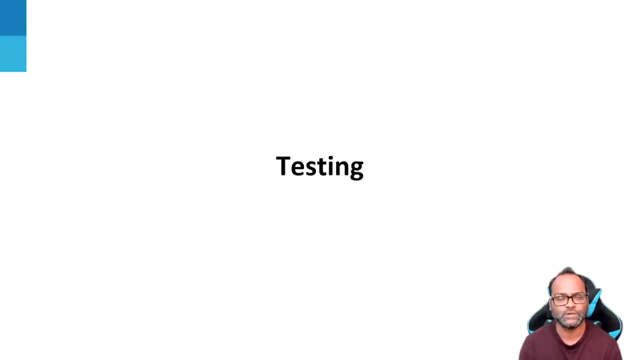 large organizations, large organizations, many large projects, as well as many, many large projects, as well as many, many large projects, as well as many large organization. it is open source large organization. it is open source, large organization. it is open source project, project, project. uh, there are some paid features which 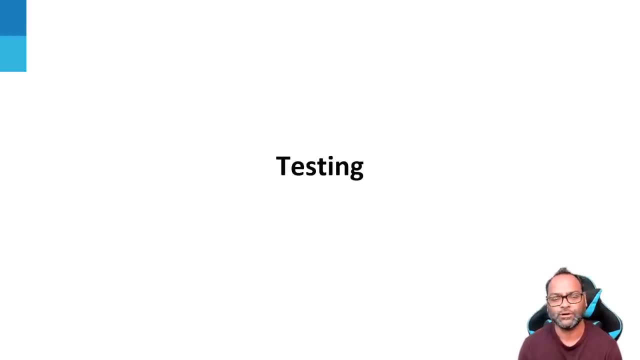 uh, there are some paid features which, uh, there are some paid features which is like dashboard, which is which which is like dashboard, which is which, which is like dashboard, which is which which probably you, you will not need that much, probably you, you will not need that much. 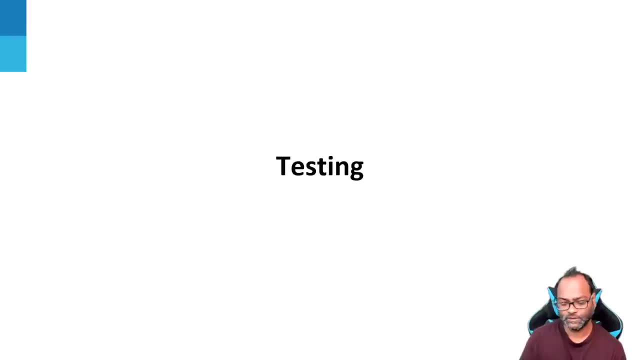 probably you. you will not need that much, but yeah, it's an open source project. so, but yeah, it's an open source project. so, but yeah, it's an open source project, so you can go ahead and use it for free. you can go ahead and use it for free. you can go ahead and use it for free. so let's see what we are going to cover. so let's see what we are going to cover. so let's see what we are going to cover here. so we are going to talk about unit here. so we are going to talk about unit. 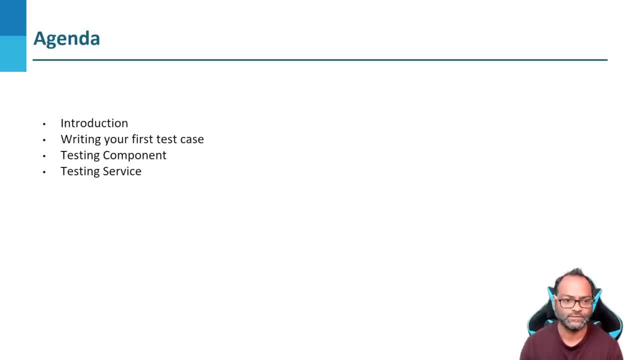 here. so we are going to talk about unit test. that's it, so we will introduce you test. that's it, so we will introduce you test. that's it, so we will introduce you to test, to test, to test, and then we'll talk about how you can. 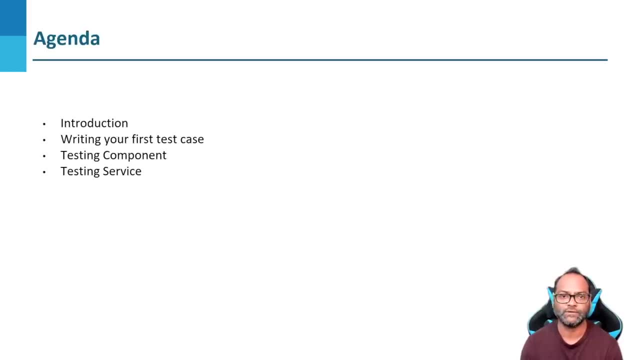 and then we'll talk about how you can, and then we'll talk about how you can write your first test, and then we'll see write your first test. and then we'll see write your first test. and then we'll see how we can test a component and how we. 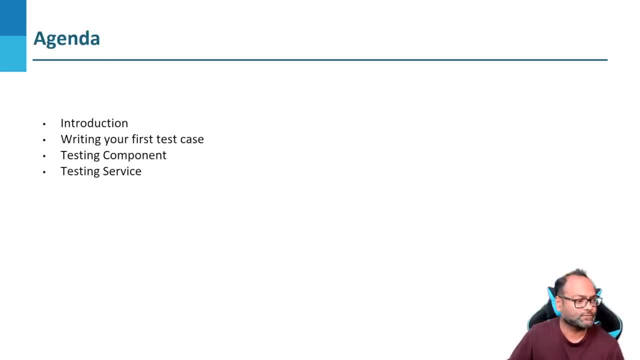 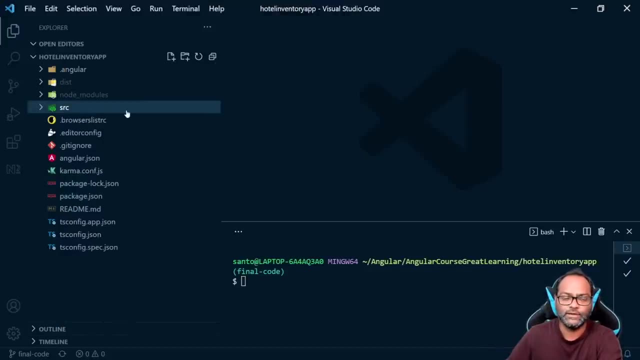 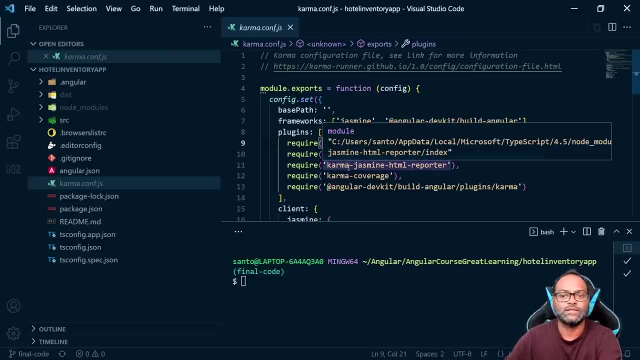 how we can test a component and how we how we can test a component and how we can test test a service can test test a service. can test test a service. this is the file which will be used by. this is the file which will be used by. 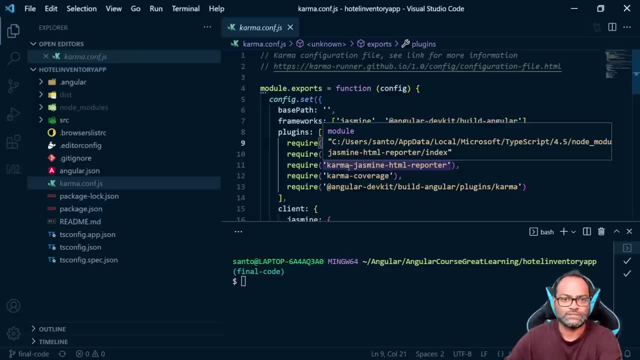 this is the file which will be used by: uh, your task runner, that's it. uh, your task runner, that's it. uh, your task runner, that's it. but we never discussed more, but we never discussed more, but we never discussed more. more about it, so, more about it, so. 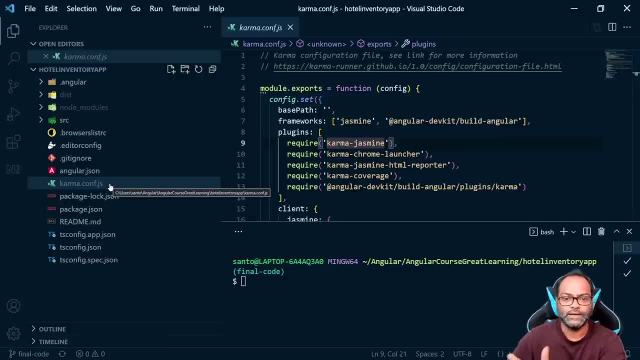 more about it. so angular uses karma plus jasmine to angular uses karma plus jasmine to angular uses karma plus jasmine to write the test case. so you can actually write the test case, so you can actually write the test case, so you can actually do ng, do ng, do ng test. you can run this command and it will. 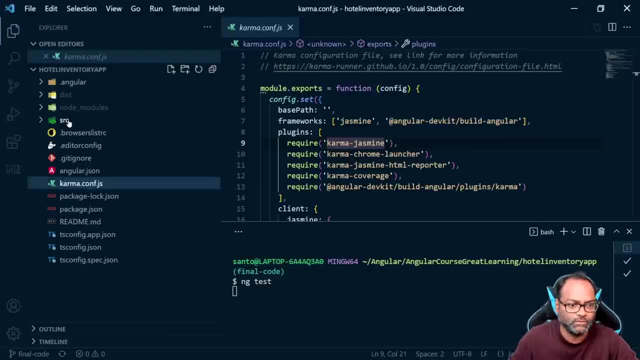 test. you can run this command and it will test. you can run this command and it will run all the run, all the run, all the test file which is available here, which test file which is available here, which test file which is available here which ends with dot, spec, dot, ds, of course. 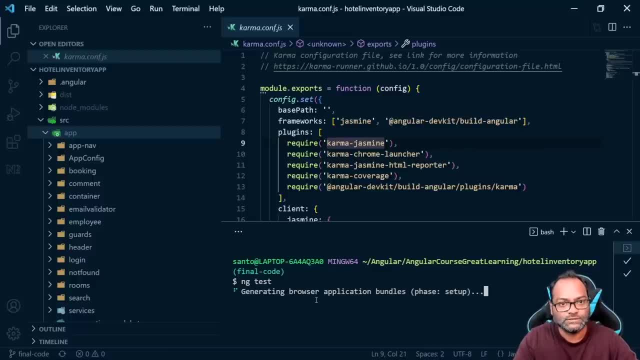 ends with dot spec dot ds, of course. ends with dot spec dot ds, of course, right now. if we execute it right now, if we execute it right now, if we execute it, you will get a lot of errors. so let's. you will get a lot of errors, so let's. 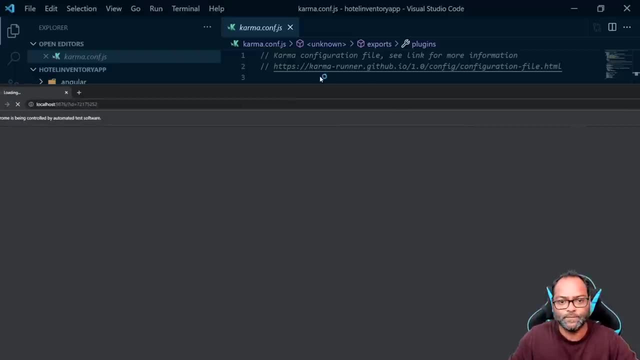 you will get a lot of errors. so let's see, i mean so it's starting the chrome. see, i mean so it's starting the chrome. see, i mean so it's starting the chrome browser. this is how it looks like. browser. this is how it looks like. 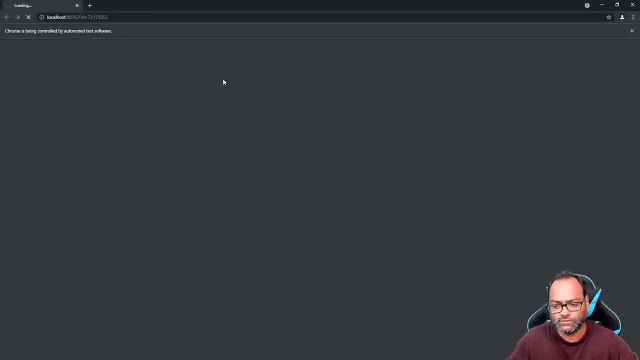 browser. this is how it looks like it does uh. there are many type of it does uh. there are many type of it does uh. there are many type of reports: uh reporter, which we have reports. uh reporter, which we have reports. uh reporter, which we have available right now. this is html. 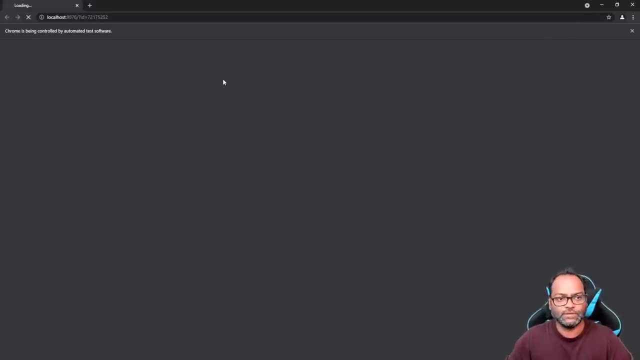 available right now. this is html available right now. this is html. reporter which uses chrome. reporter which uses chrome. reporter which uses chrome and it will open everything in chrome and it will open everything in chrome. and it will open everything in chrome and it will show you how many tests are. 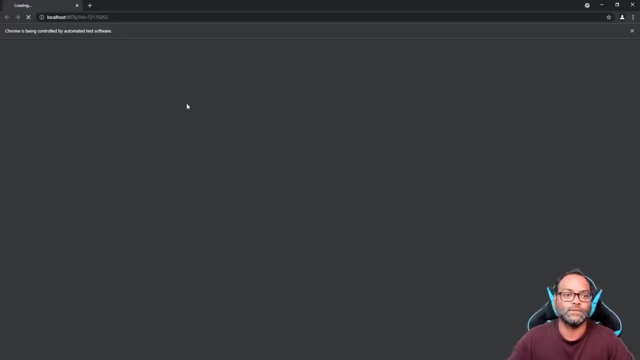 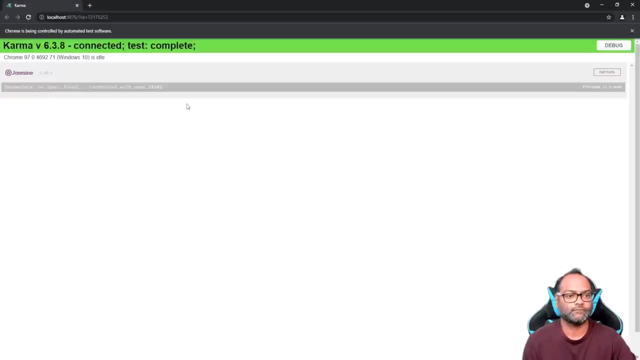 and it will show you how many tests are. and it will show you how many tests are getting passed, how many tests are getting passed, how many tests are getting passed, how many tests are getting filled, getting filled, getting filled. so let's go ahead and see that. so it says incomplete: no specs found. 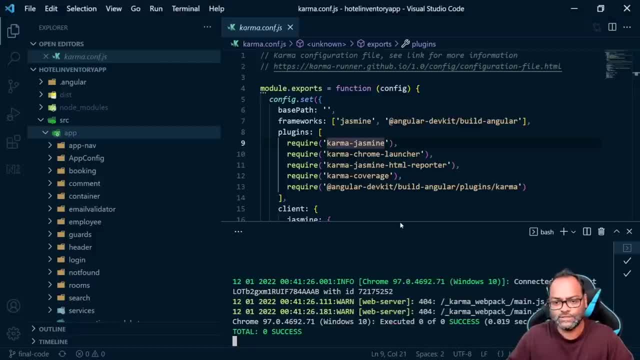 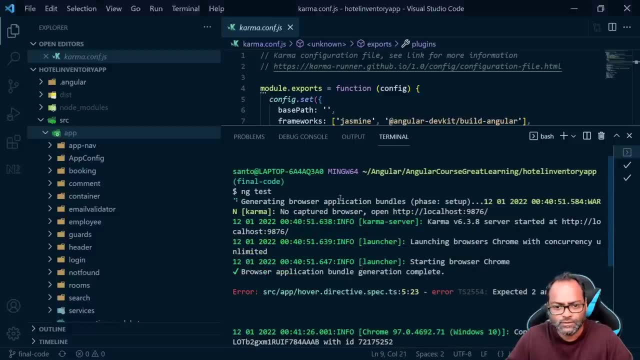 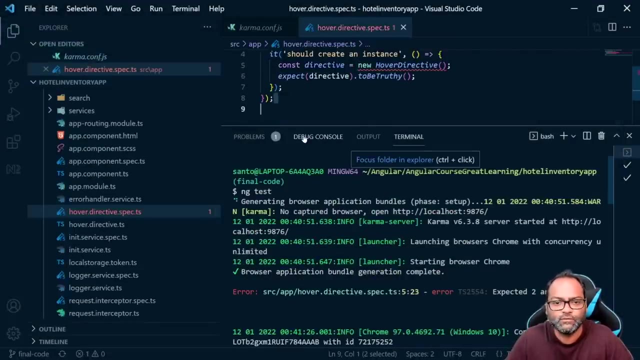 so it says incomplete: no specs found. so it says incomplete no specs found somehow, somehow, because there are some errors, right, so you can see there are some errors. which is making this? so let's see what this error is. it says expected to argument right now. what we will do is we will 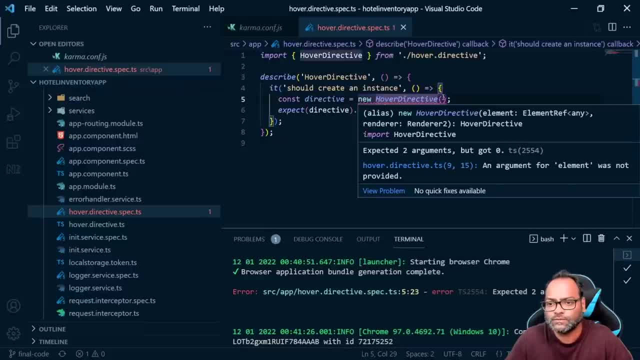 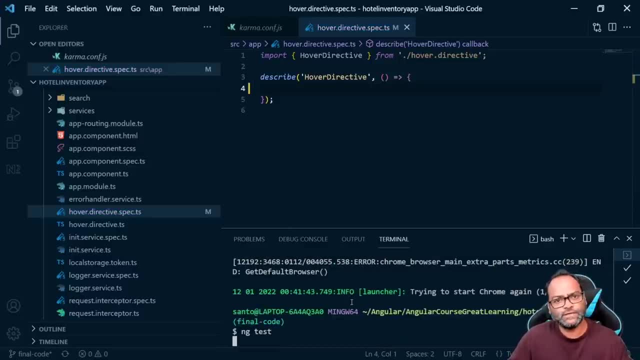 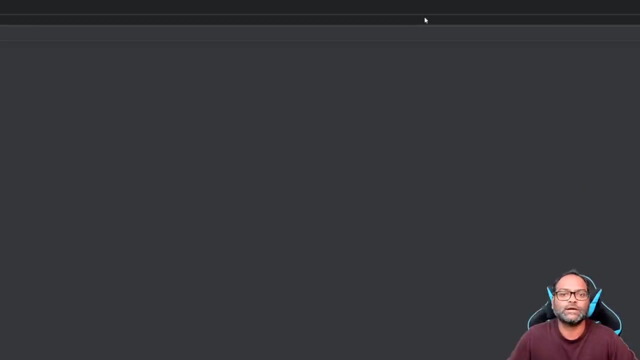 just remove this and let's see- so at least we get the uh feel right- how your ui looks like once you run the ng test and how your report looks like. sorry, testing is a whole topic all together. so it says there are, because there are different tools which are available. so we are not. 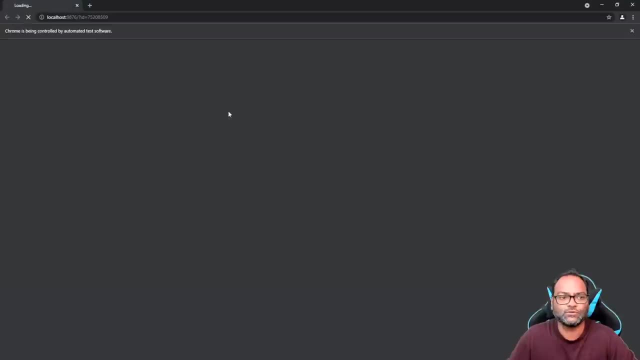 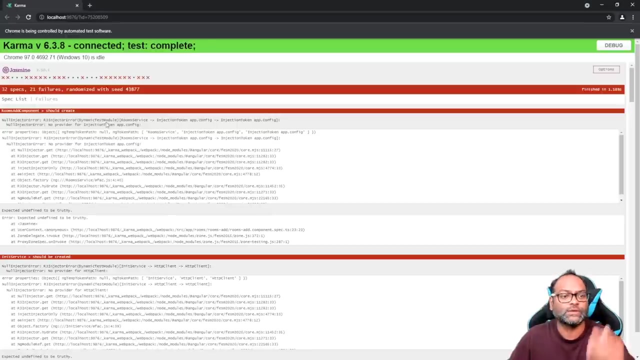 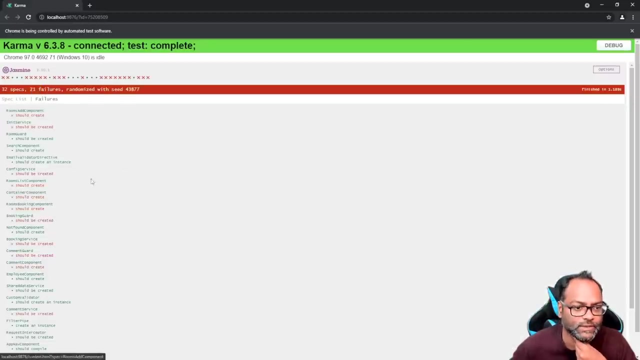 going to go into that much detail here. it will just we will introduce you to the testing and let's see, uh, probably there are no errors you can see right now. so, uh, there it says there is 32 specs which, out of which 21 is failed. so you can see spec list, the green ones. let me just 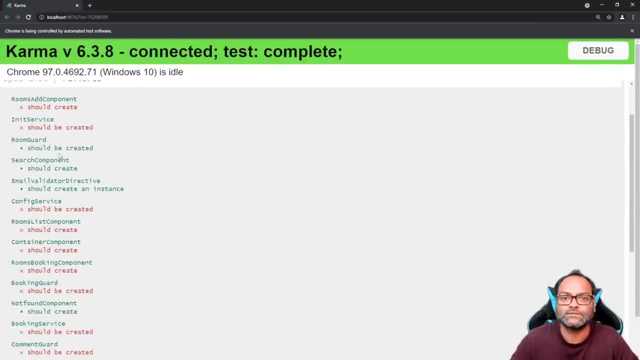 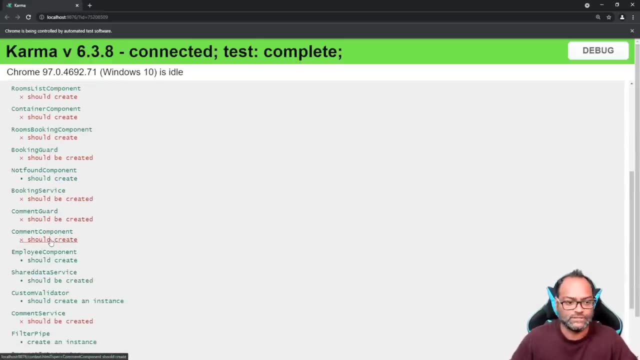 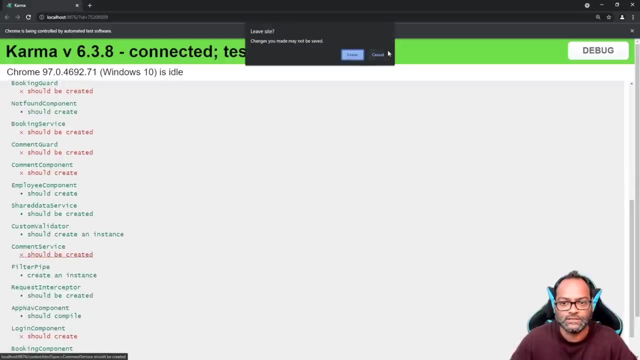 zoom in. so this green ones is successful and this red ones. of course, it shows that this, this is a failure. so this is how you can figure out, okay, which test is getting passed, which which test is getting failed. so here in command service should be created so you can see, okay, it's not. 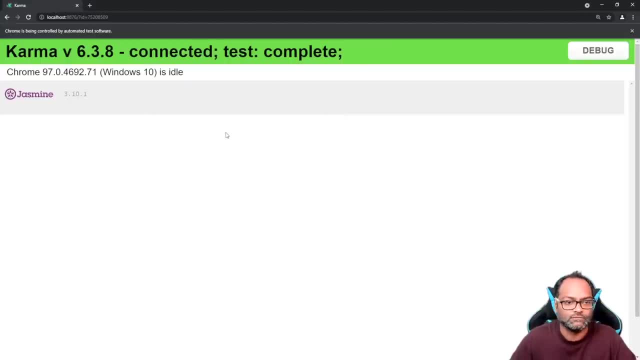 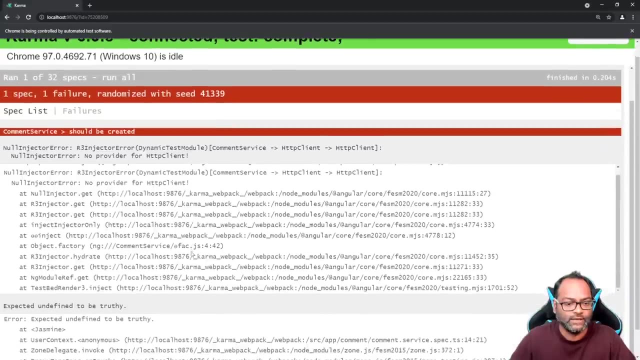 uh, it is giving me error right now, so you can just click on the test as well to see what's going wrong. so it says okay. uh, it says no provider for this to be client. so while testing, we are not providing the certificate line module. so that's the problem. so we can fix it. so let's see, let's. 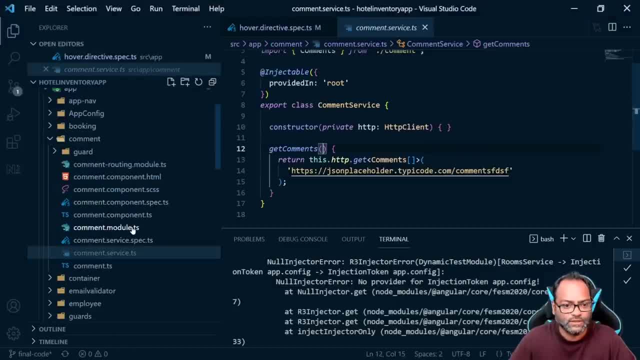 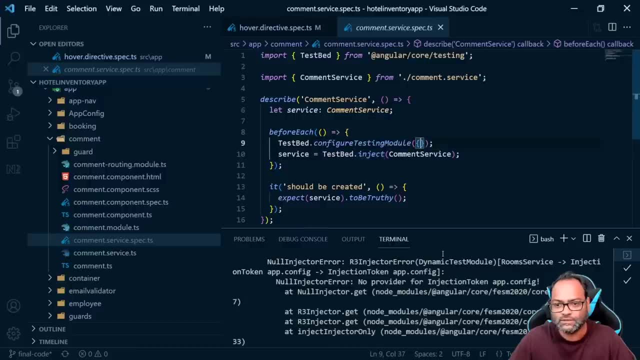 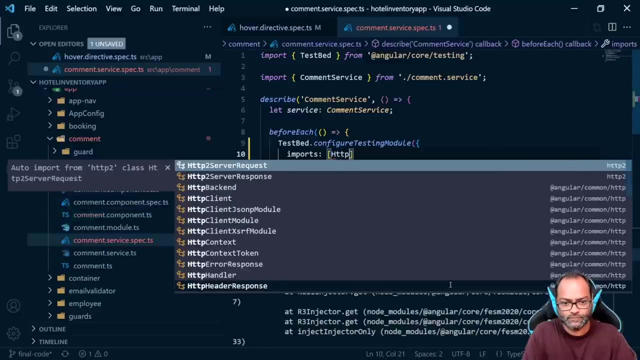 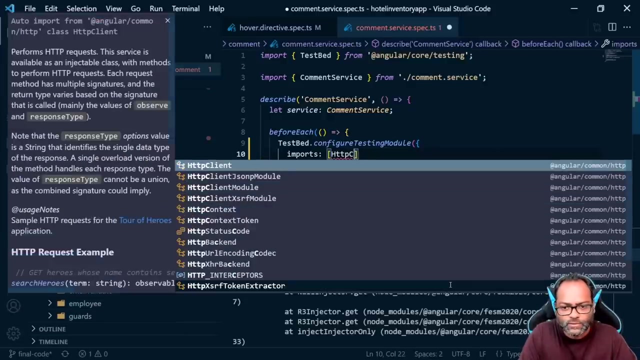 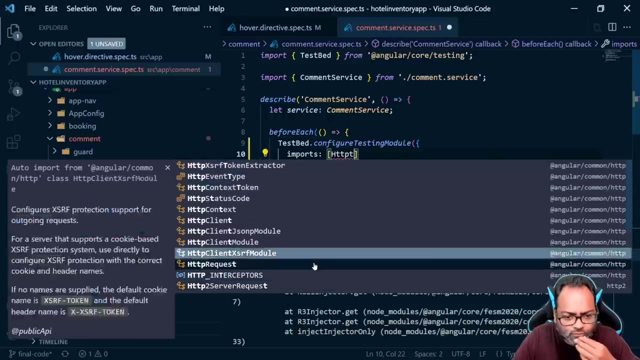 try to do that. so here in command service, uh, servicespec, we can do test, configure testing module and then we can say: import uh http client testing module. so there is something known as specific client should be testing. what is that called http client module? let's look at client. 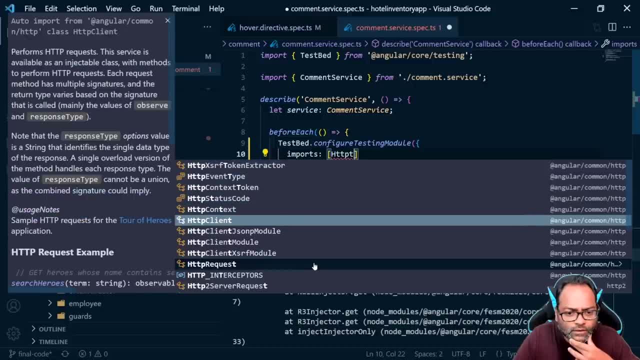 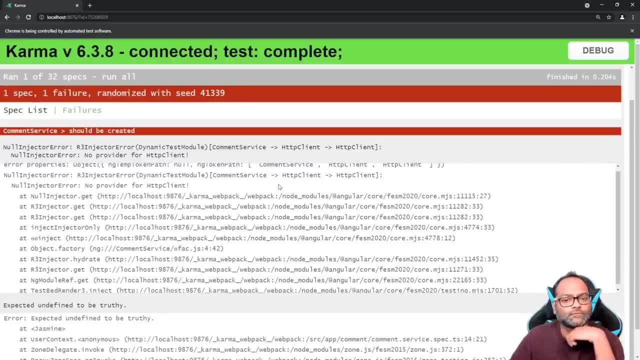 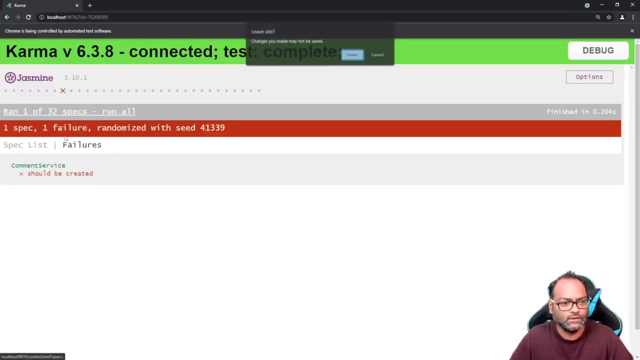 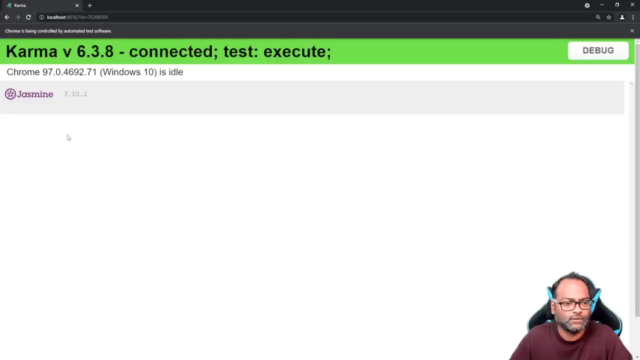 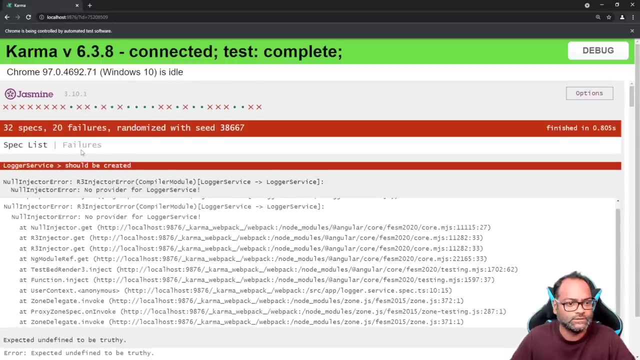 okay, let's try to pass http client module right now and see, because this http client of course exists inside http client module. so, okay, uh, let's see spec list. okay, it's still being failed. so let's go to the spec list and see comment and let's see failures. and now you can see there are 20 failures. so earlier there was 21 failures. 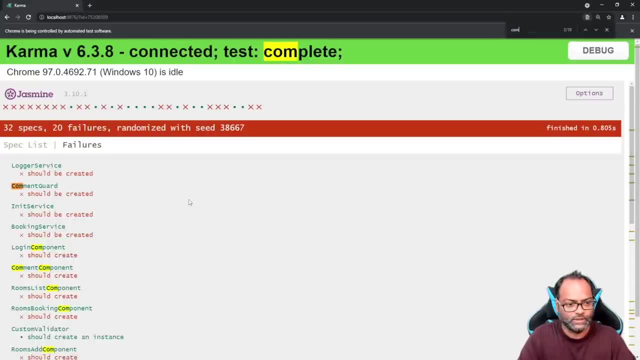 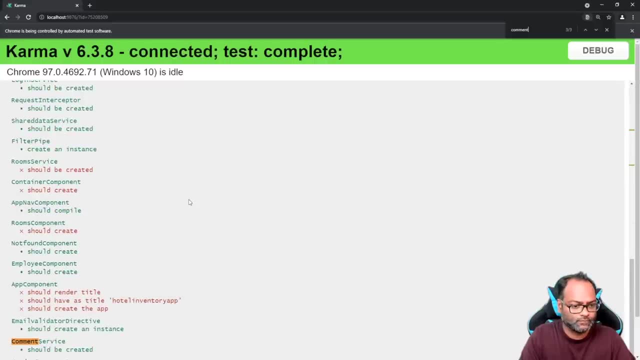 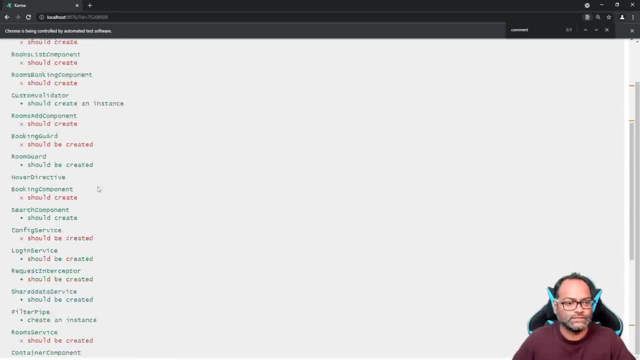 so probably, uh, let's go to spec list and see comment so you can see comment service created past. but uh, i mean, this is just to show you how the report looks like and how you can see, uh, what is the error. you can just click on this line and it will. 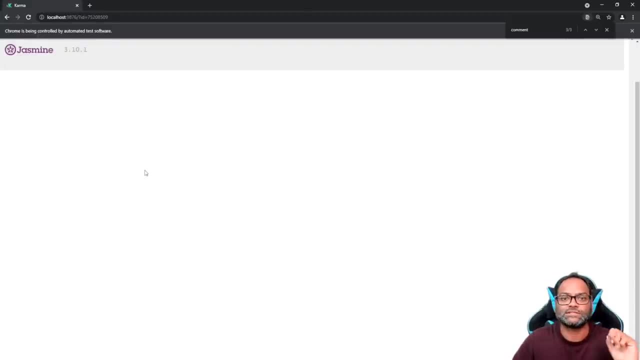 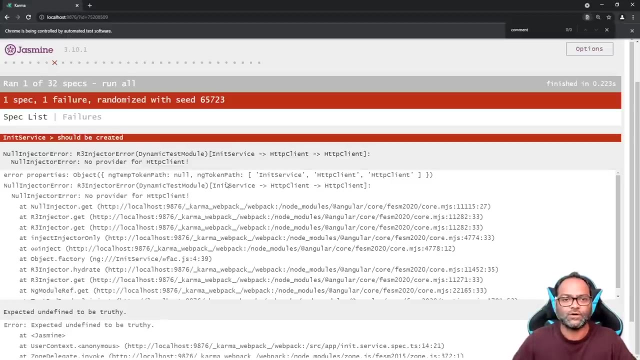 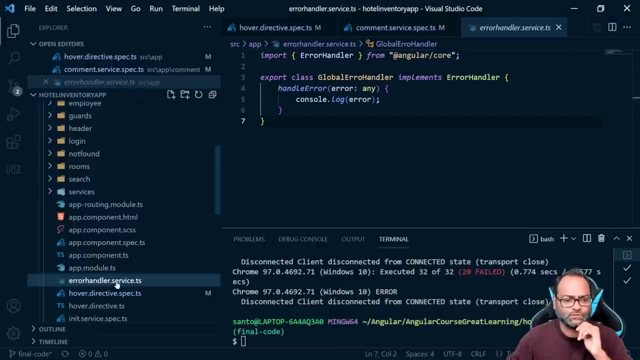 tell you, uh, that, okay, this is the actual error and why this particular test is getting failed. so let's go ahead and try to write a little bit of test cases for a component and a service. see how we can write a sample test case using jasmine. so the idea is to give you uh. 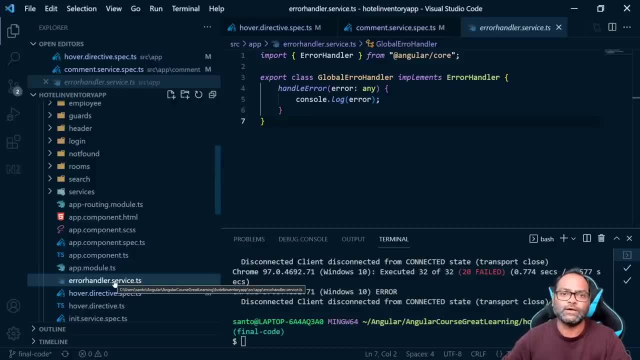 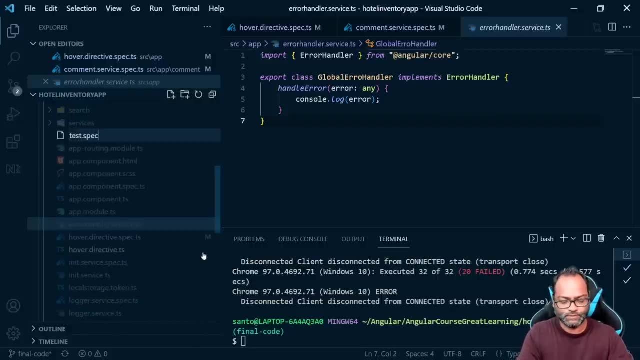 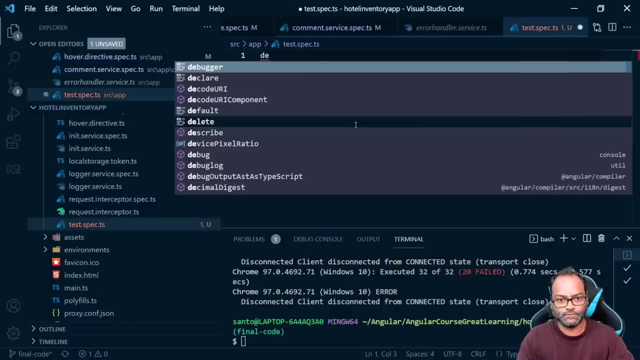 sorry. so, uh, the thing is, uh, it will give you a little bit idea how you can actually write jasmine test cases and let's create a test file. so i'll say: this is test, dot, spec, dot, ds. so here, uh, generally what you do is you write a describe block where you will describe that. 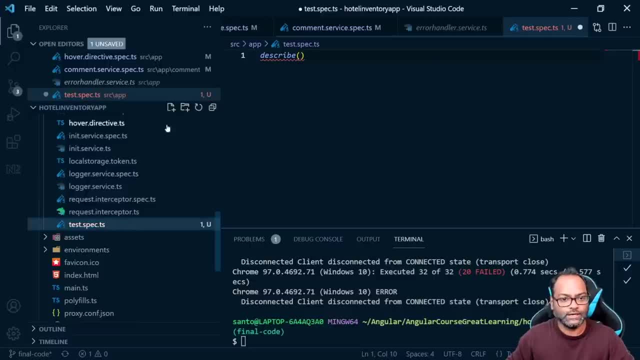 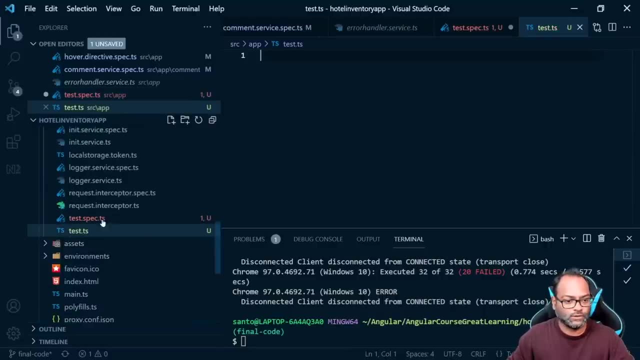 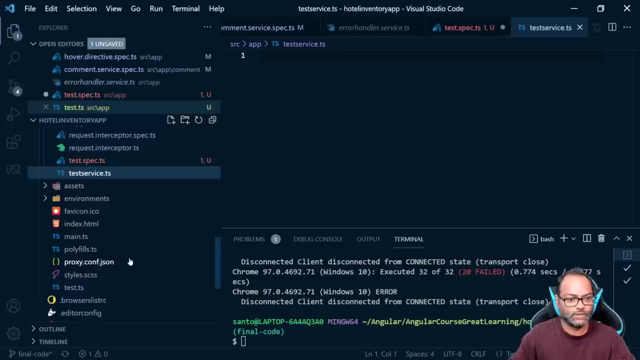 what you are trying to test, and to do this i'll create a file as well. so i'll say: this is test dot ds. so let's see if there is another test of ds. yes, so i'll say this is test service dot ds. so the first thing is, you will write that. okay, let's. 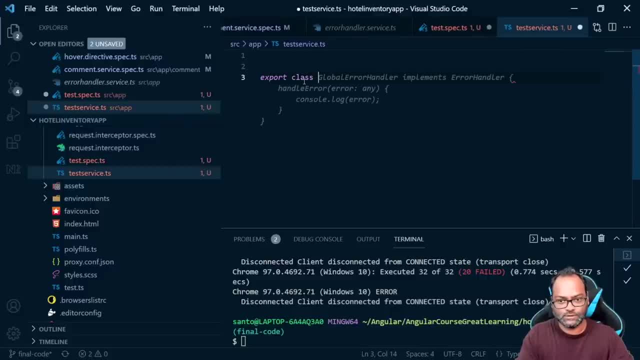 let's add a class which is calculator class and then we will have some functions which will say one is add and then we have subtract and multiply, okay, so there's a few few implementations which we have inside this calculator things. let's go ahead and see how we can test it. so the first thing is we need to import what we are trying to test. so 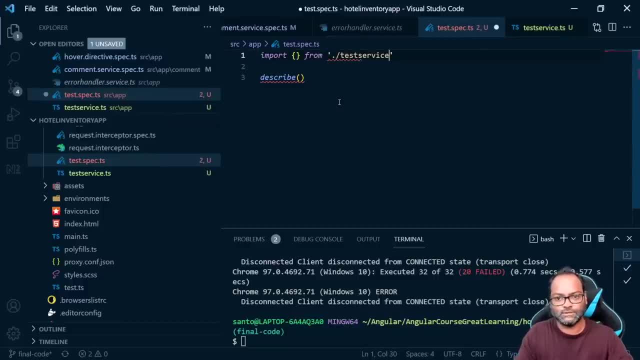 we'll say, okay, we are trying to test service. so i'll say, okay, this is describe. and we'll say, this is test service. and we'll say, okay, this is where we are writing the code, so your tests should look like a story. so we are saying, okay, we want to test this, uh. so in describe we are saying, okay, 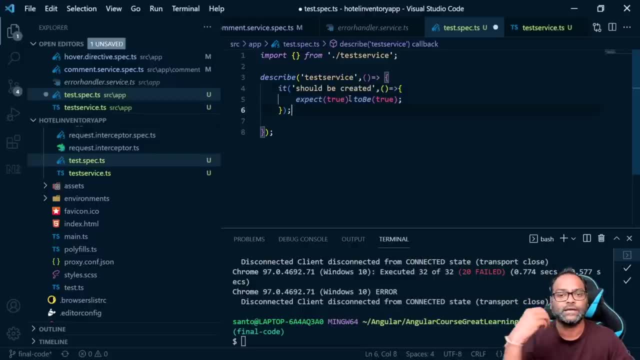 we are trying to test this particular service and then you will write the steps, what you are trying to achieve. so first is of course i will say: uh should add two numbers, right? so this is uh one of the tasks or one of the test case, uh for our particular, this particular service. so 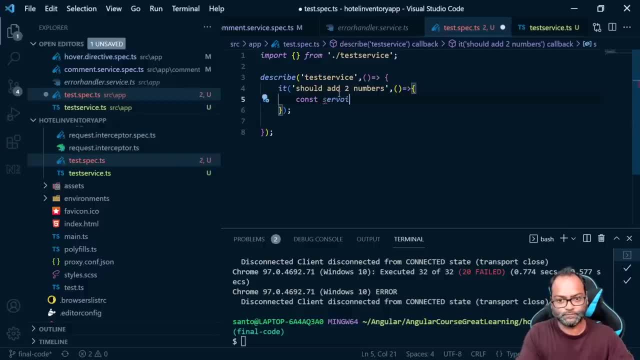 i can say, okay, const uh service is equals to new uh test service, which will take it, import it from here. what's the name? not calculated, sorry, okay. so we uh created a new calculator service and then we can do something like this. so we can say: expect, so, uh, we have to write. 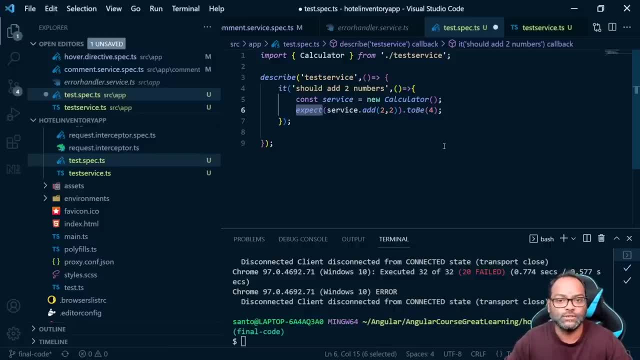 a new calculator service and then we can do something like this so we can say: expect, so uh, we have to write a expectation that what this test case should do. so we are saying that, okay, whenever we run this test case, just go ahead and add this two number and the answer should be four. that's our expectation. 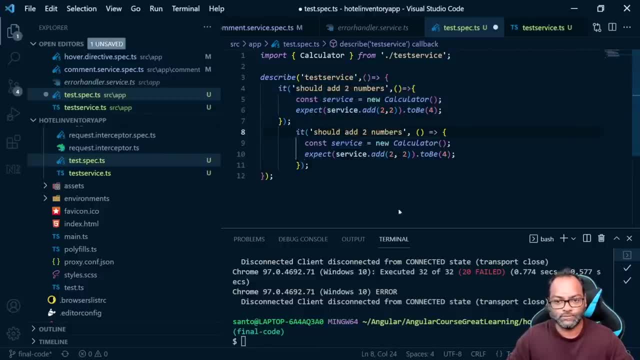 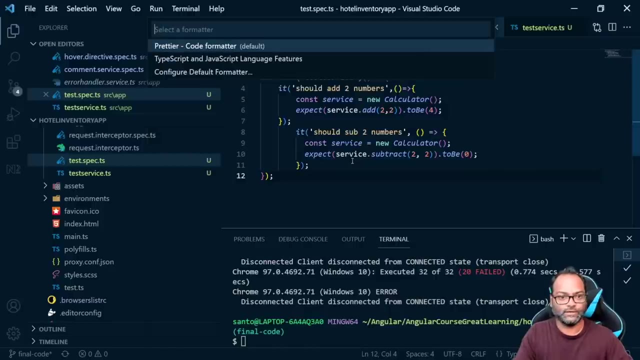 so similarly i can just do it for uh should subtract two numbers and then we can say: okay, this is subtract, and uh, we'll say: answer should be zero. let's go ahead and run this, so we can just do into test and it will go ahead and run all the test case, because 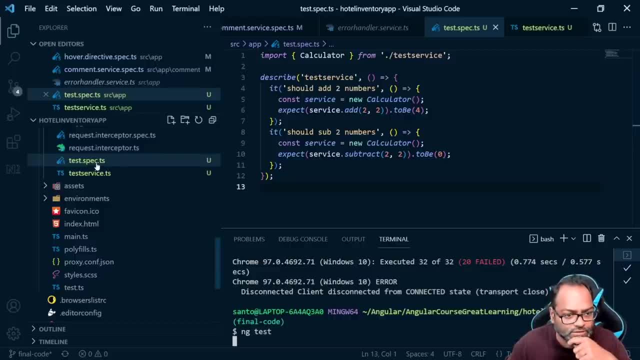 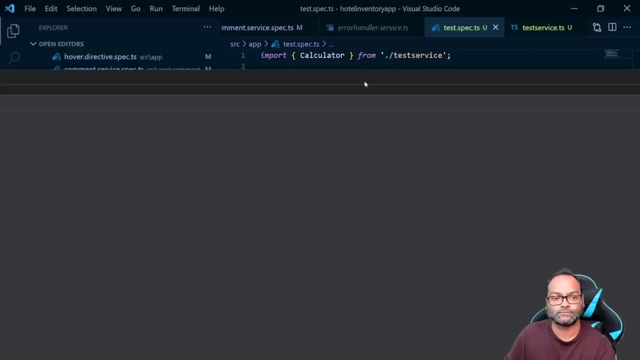 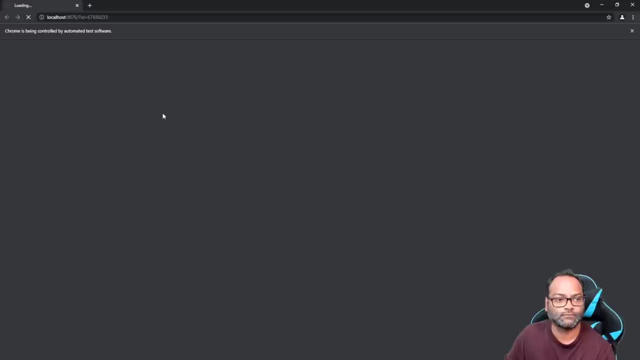 this file matches the format, which is dot, spec, dot, ts, and it will open it in browser. so a lot of projects also use something known as uh, just for testing, which is a little bit faster, but right now it's not compatible with angular 13. that's one of the 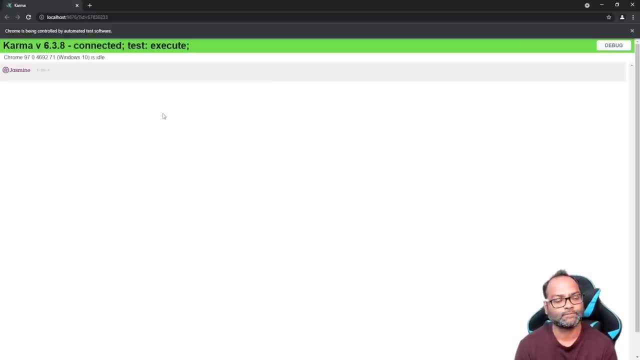 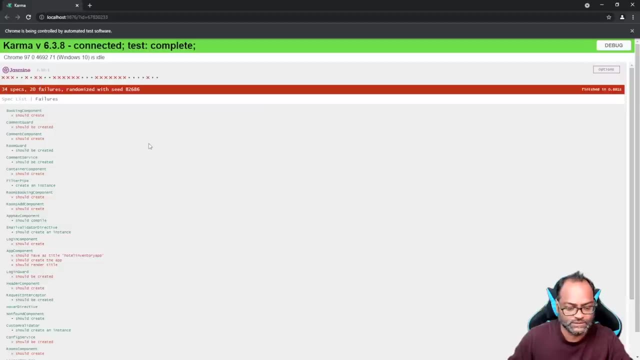 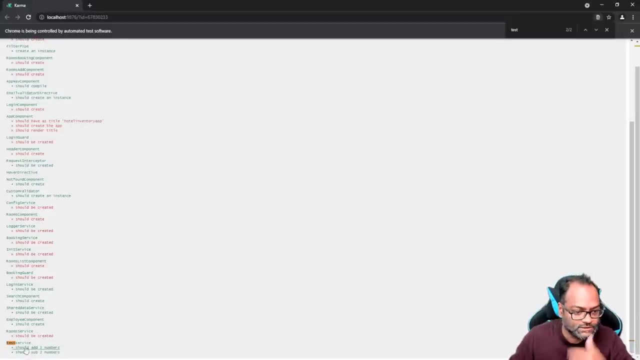 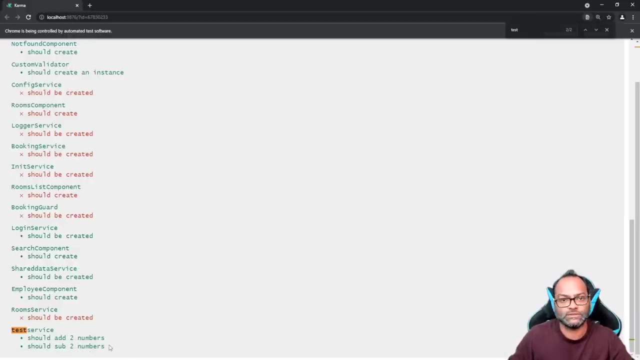 issues. okay, so, uh, we are saying we are seeing now there are 34 specs and let's go to spec list and let's see calculator one. oh, sorry, we said test service, right, yeah, so you can see, uh, this two, these two tests are getting passed, so should add two numbers and should subtract two numbers. it's. 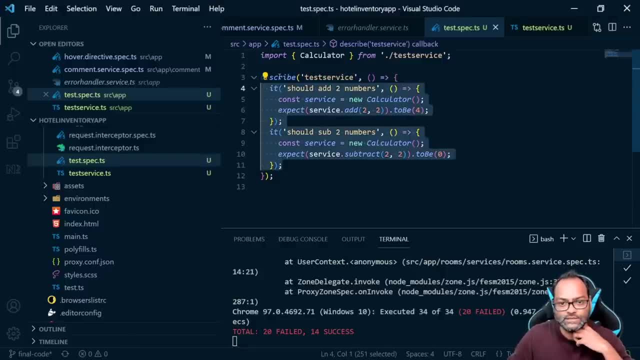 getting passed. so it should add two numbers and should subtract two numbers. it's getting passed. so this is how you actually will be writing the test: start with describe block and then you will be writing the story that, okay, what now? this this should do. so it should add two numbers, it should. 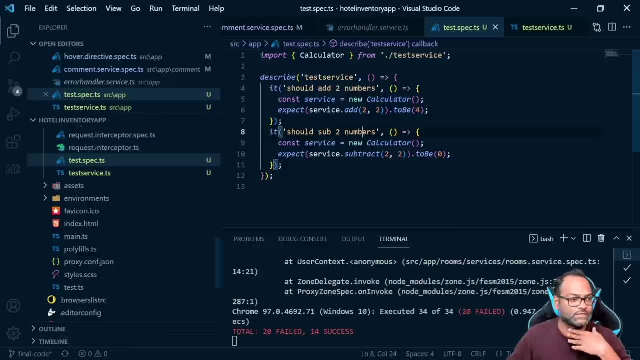 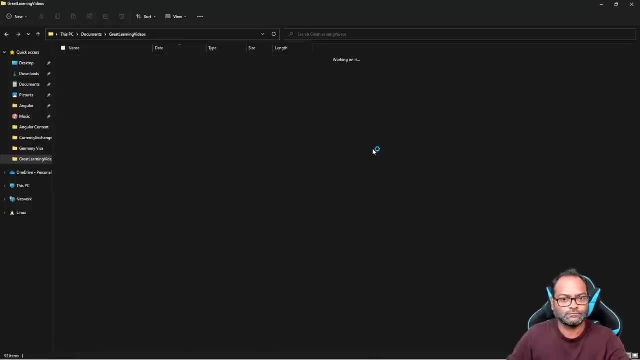 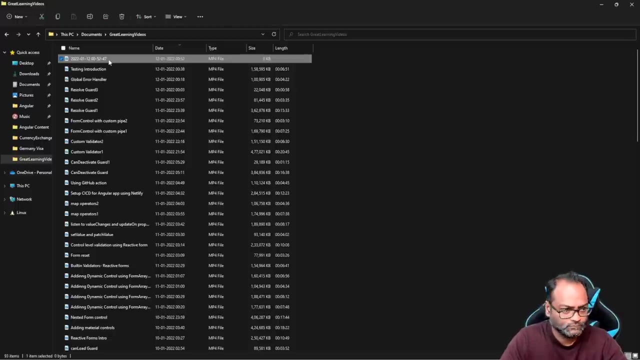 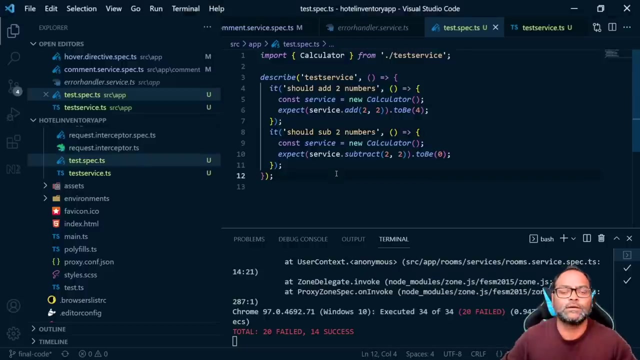 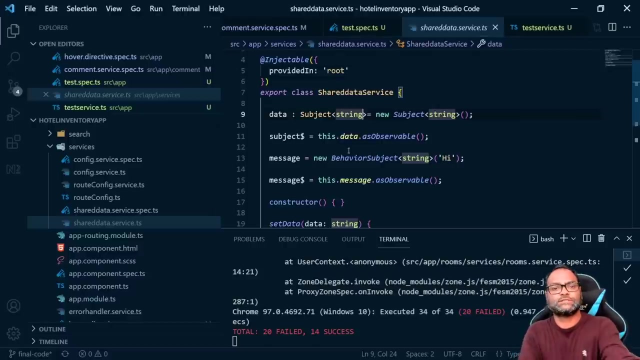 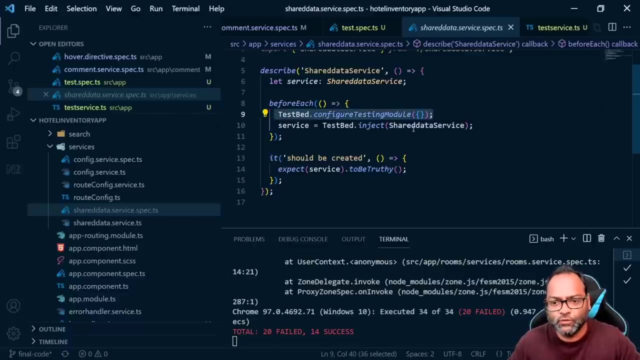 subtract two numbers. so this is a sample test case. let's see how we can test our service. so here let's try to do uh service. let's try to test this shared data service right? so we already have a spec file available here and there is something known as configure testing model, which we don't need right now. but let's see. 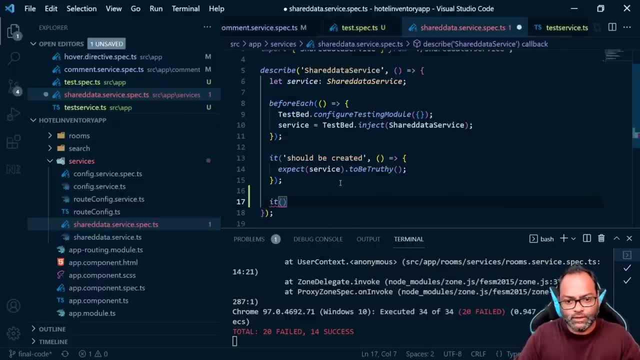 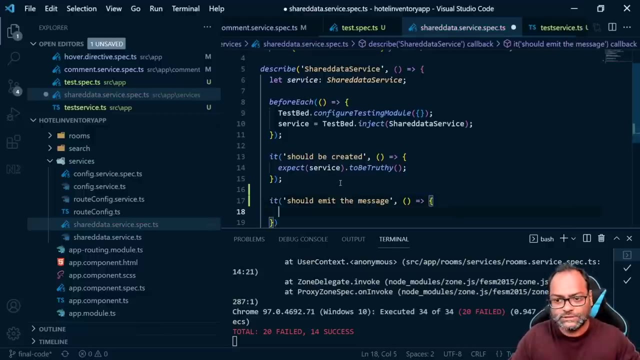 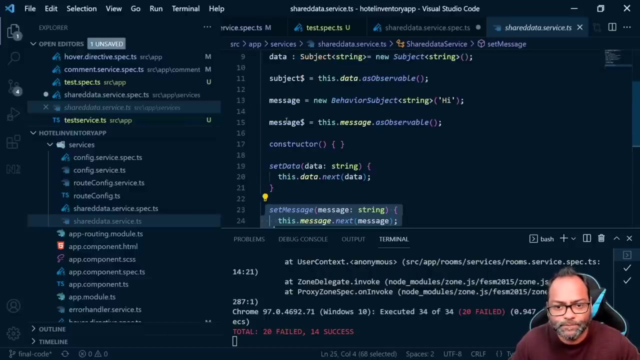 what we can achieve using this. so here i will say: it should emit the message, basically. uh, what we are going to do here is we are going to test the send message, right? so? if you remember, in shared data service we said set message, which actually emits a new message, right so? 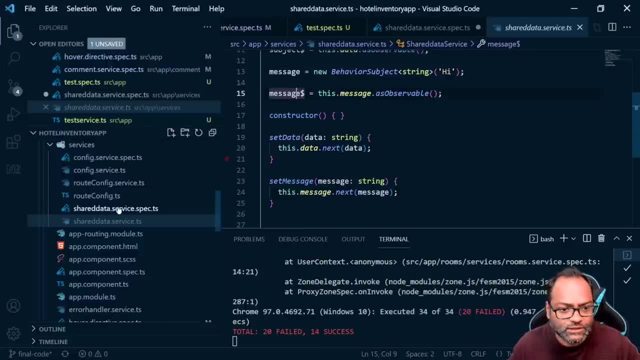 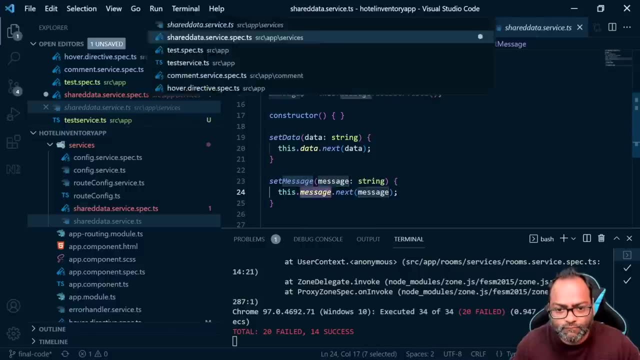 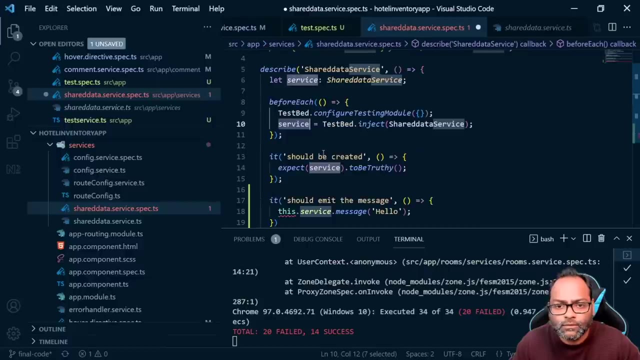 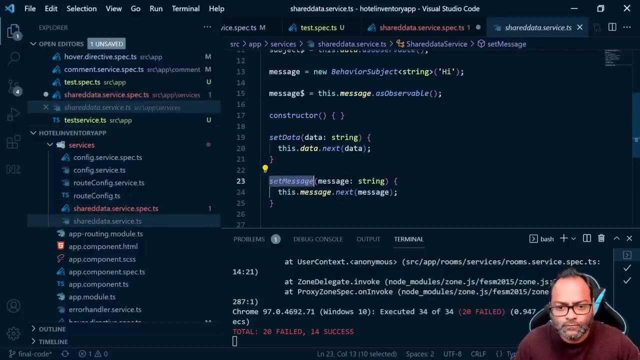 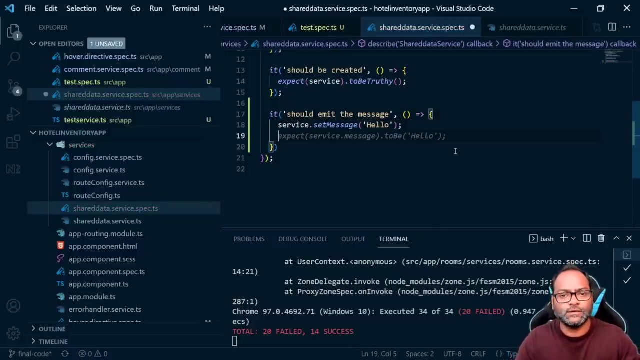 one, sorry so, which emits a new message. so we will check this. so here we will do this: dot our service dot set message, okay, and once we do this, the expectation is we should get a hello message in this stream. so we will do something uh simple right now so we can say: message dot subscribe. 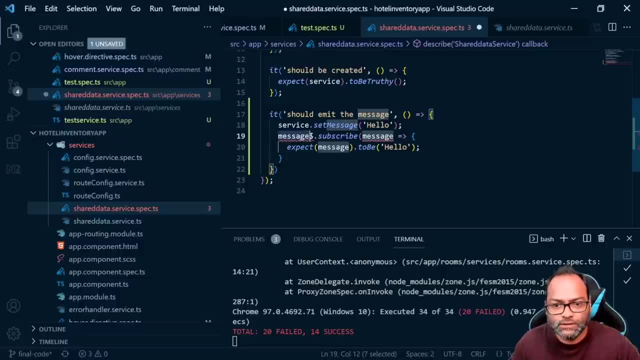 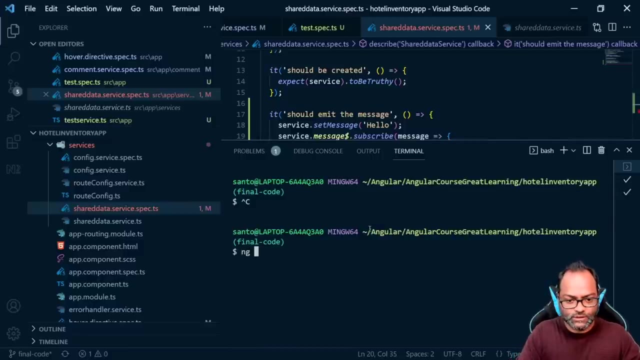 and then we can say: uh, expect this message to be hello. so sorry, this will be service dot message stream. and then we'll say: message to be hello. and now let's stop this. let's disconnect the data from here. let's just go just a little bitтак. capture this file now. we will do a performance. 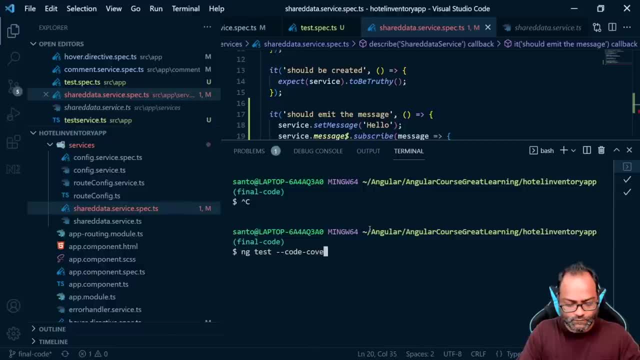 test again. we have a lot of tasks, so first we have to check when this application is searched. so if i am hyphen, hyphen output test, we will also see something. uh ng test, hyphen, hyphen code coverage. let me tell you about this as well. 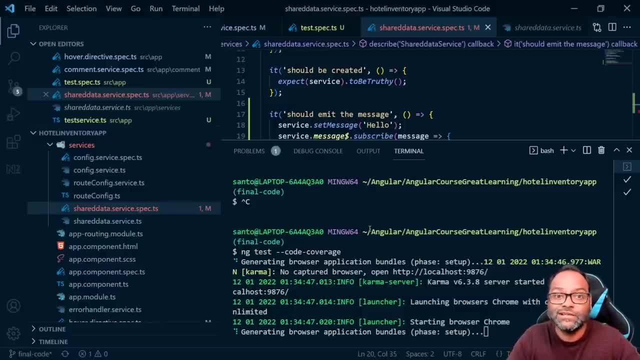 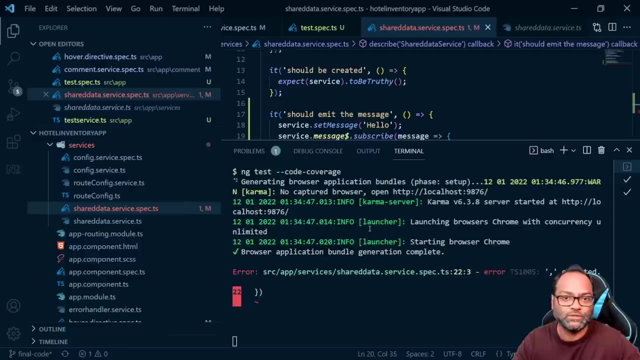 while testing you can also test how much code is being covered by your test cases. so there's no hard rule i would say. i mean it depends upon how much code you think is worth testing. can uh go to 80 code coverage? i think it's. it's a false uh alarm, i would say most of the time. 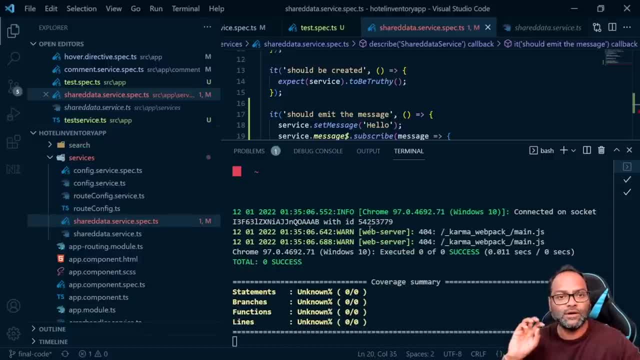 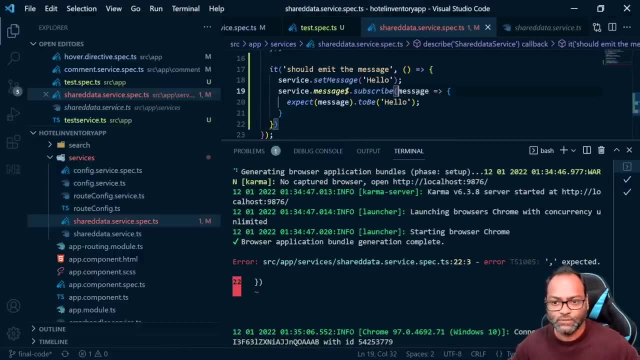 you may get a false alarm. the thing is, you should concentrate on what logic is worth testing. i mean, do you think this, this should be tested? if it is not, i think it's okay to skip. so here let's see what is wrong. i think there is an extra bracket here, so 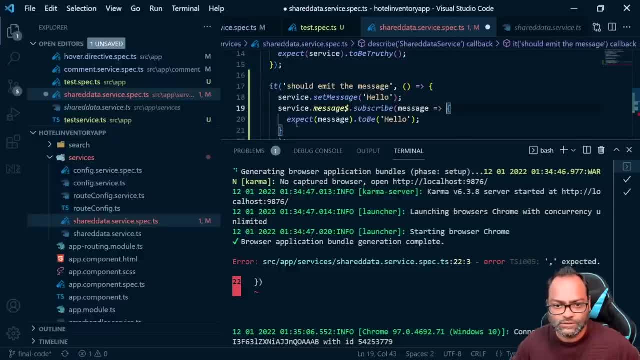 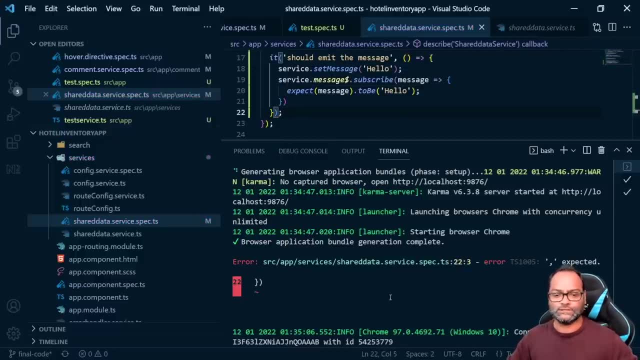 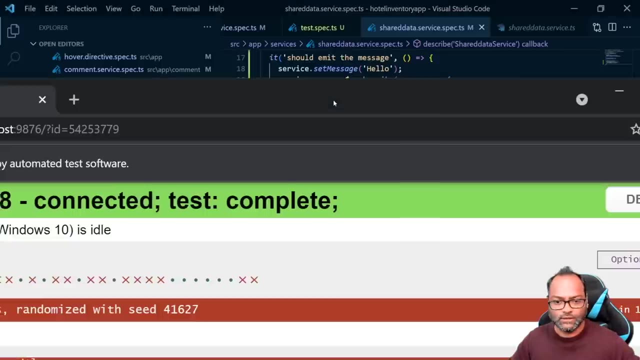 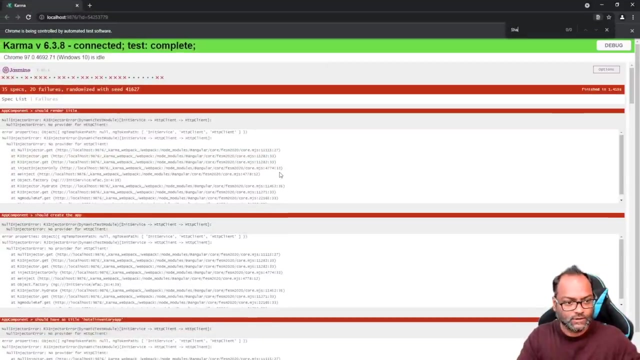 it's a message, then it should close here, and then we have the outer one and close. let's see. so it's completed now tests are running and you can see. uh, the one which we are looking at is shared. let's go to the spec list first. 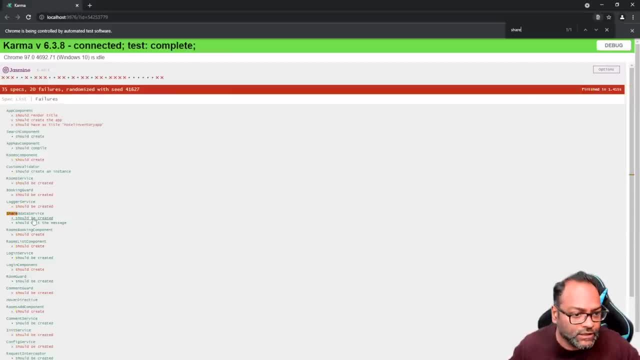 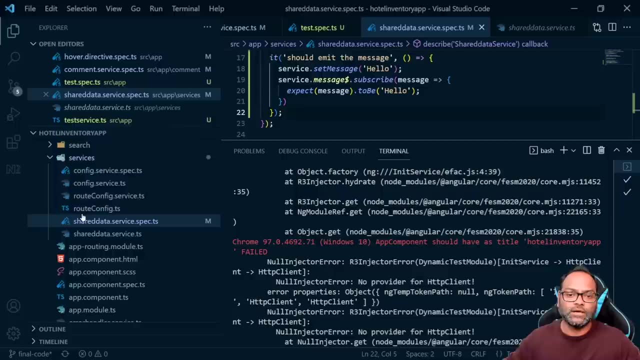 shared, so you can see shared data service and it says this was successful, so should emit the message. it means: uh, what our expectation was that whenever we send this set message, whenever we call this set message, it should go ahead and the message whoever has subscribed to the message. 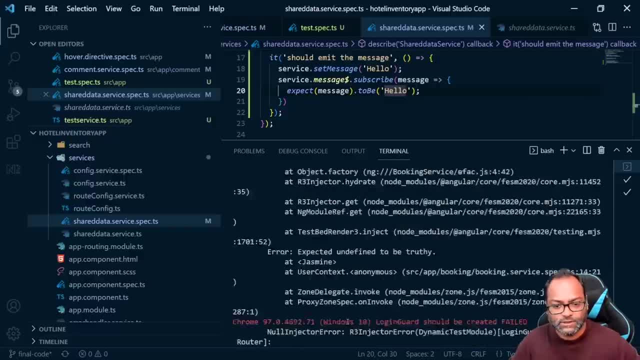 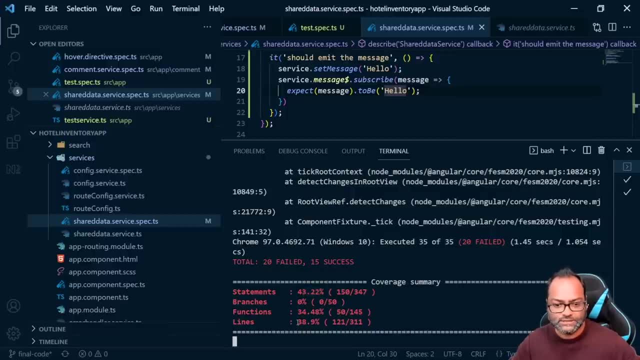 should get this hello message, and that's what we tested and it worked. so here you can see. uh, the code coverage is, of course, right now pretty bad. so we have statements, which is covered at 43 lines, 38 percent of 9, 38.9 of lines are covered, and then we have functions, which is like 34. 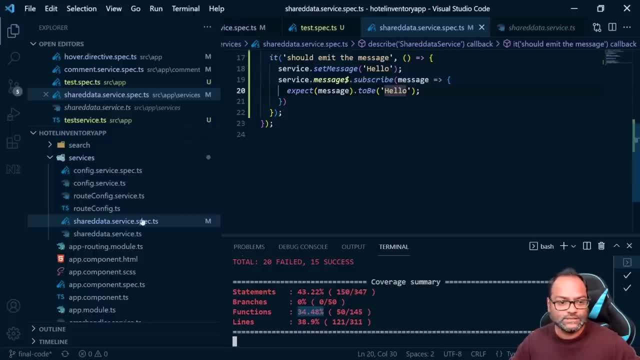 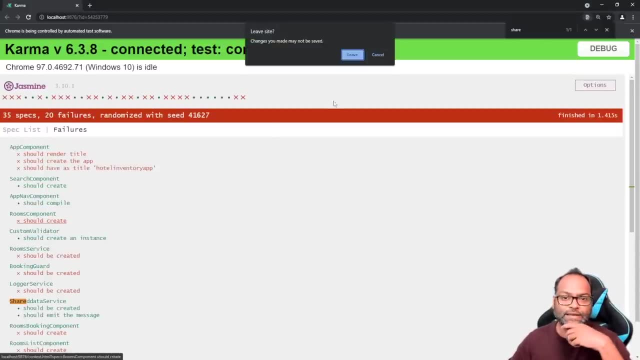 covered. so, uh, now let's go ahead and see an example of a component. so we already have some components which is getting failed, right? so let's see rooms component should create. now let's see how we can actually fix this particular test case and you can click on error. 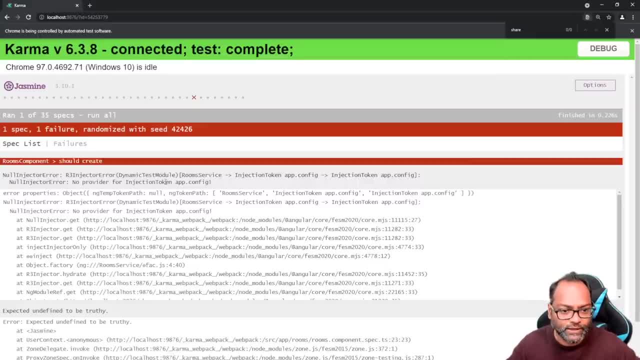 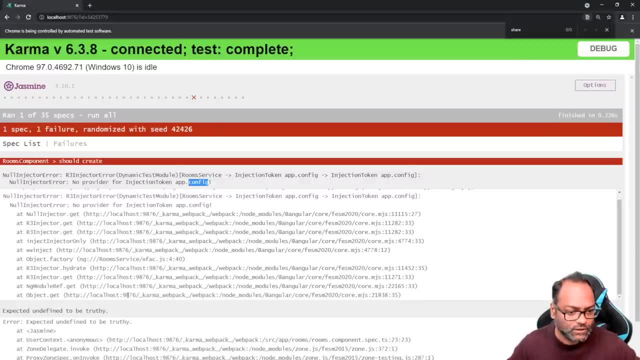 and see what is the error. so it says, okay, the thing is you need to provide an injection token. okay, let's see how we can work out when it's not working with this. there is a few, there are a few errors, so let's see, let's go to. what was this? 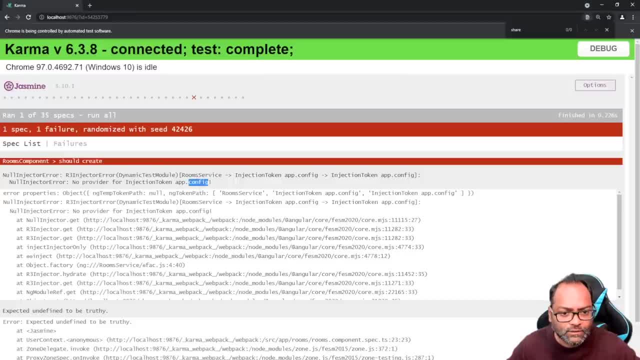 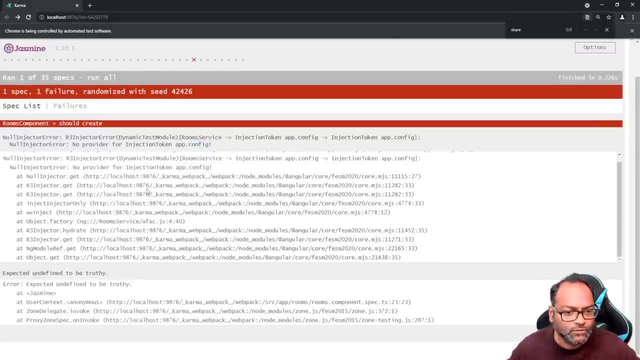 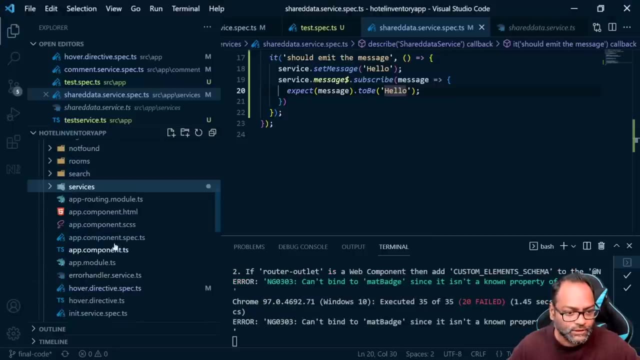 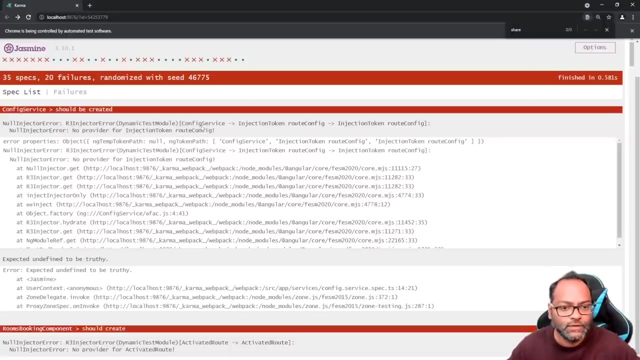 room, not room service. but which component was this room? it was it rooms component. let's, let's go back. i think it was rooms component. so let's go back to rooms componentspects. okay, so we have this. it says: okay, we, we have not provided the config service. 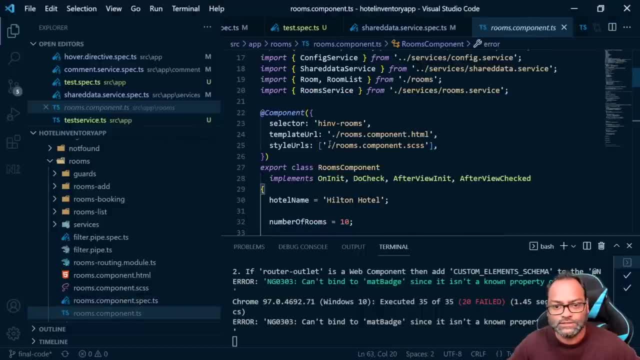 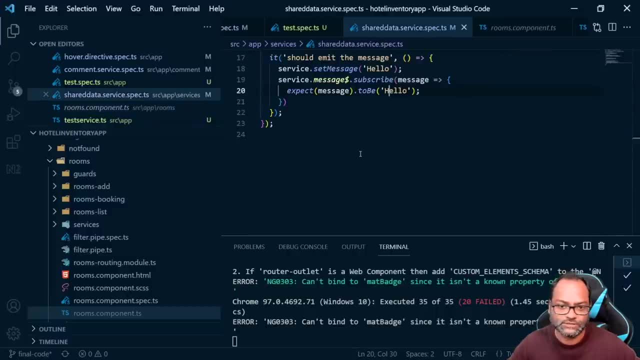 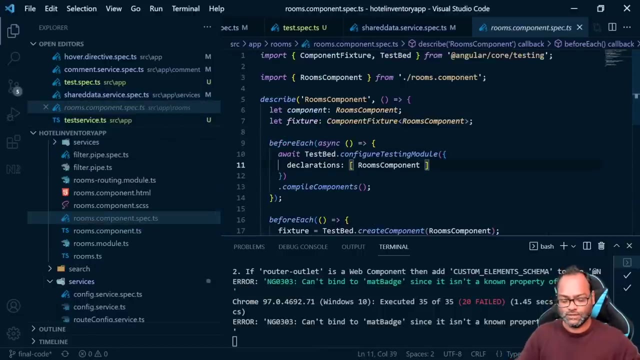 because, remember, you have to go ahead and provide all the services which your component is using right now. so it uses room service, it uses config services, you, it uses shared service. so we can, uh, go to sorry, we can go to this and here we can add providers. so we can say: okay. 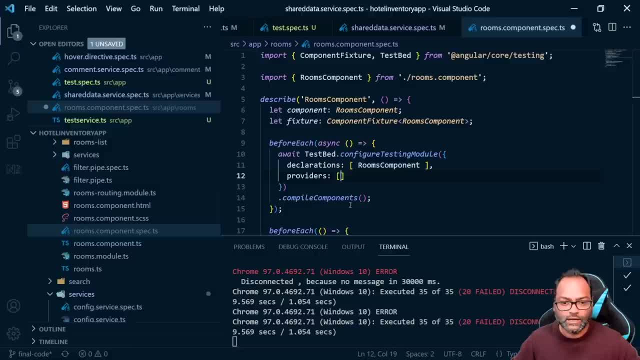 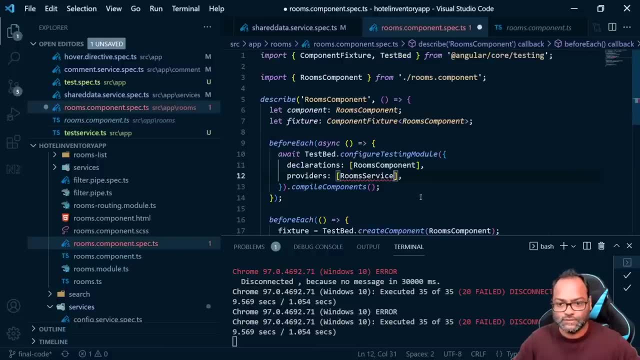 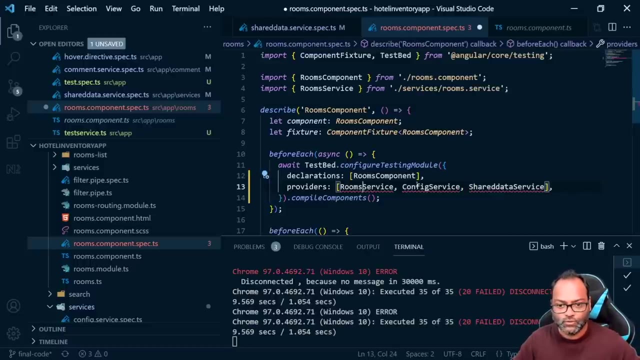 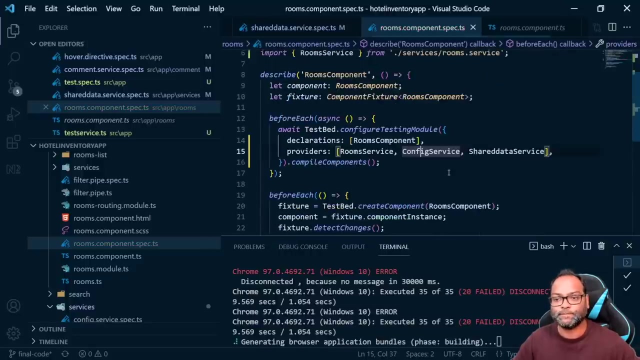 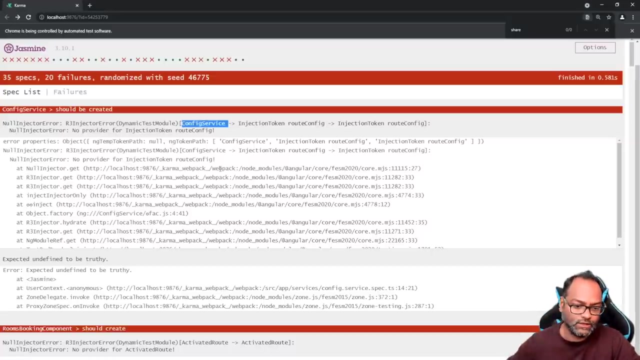 providers array and let's add all those providers which are being used. so we have room service, we have config service and we have a shared data service, and let's import each one of these and let's see now, uh, let's see what's the error we are getting right now. it says also: activated route is not provided. 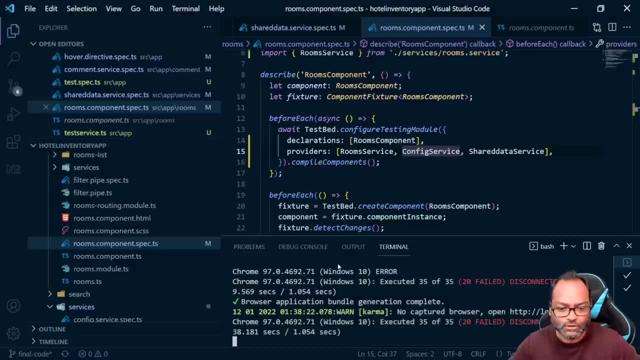 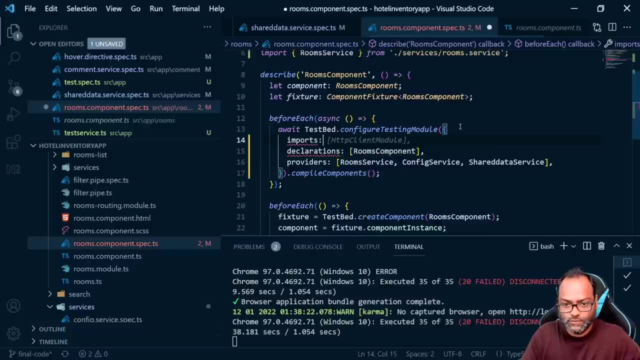 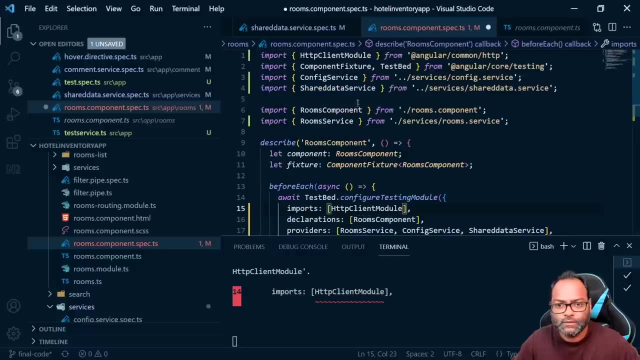 and sdp client. we'll see some uh. the errors will be gone one by one. so it means we need uh to import imports. sdp client module: let's see sdp- i think that was testing as well- and sdp, we can use the testing module rather than actually original module. we can say okay: 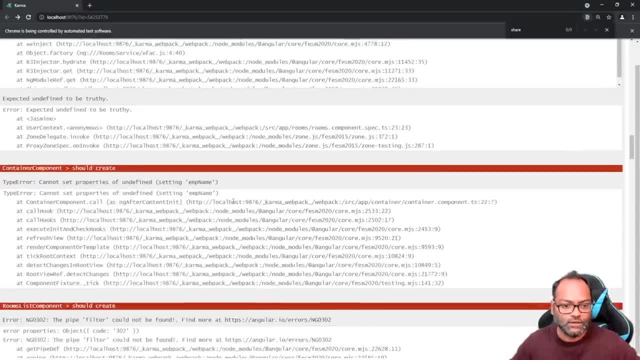 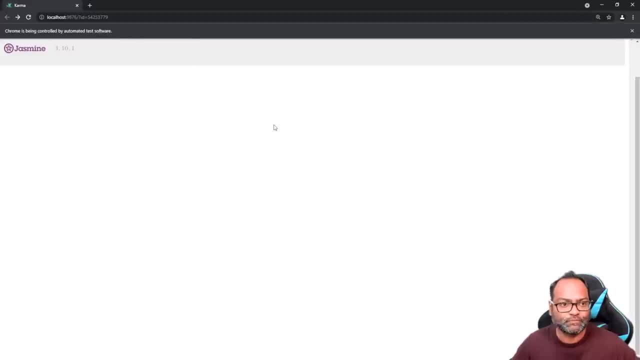 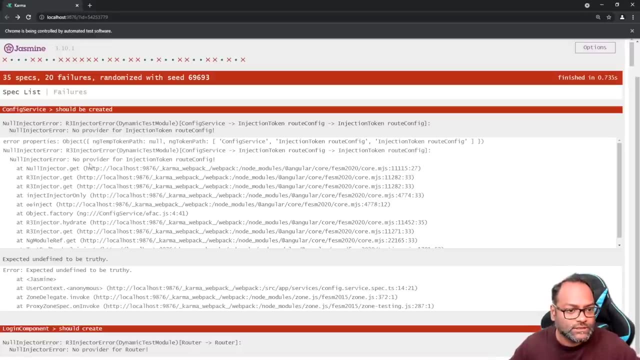 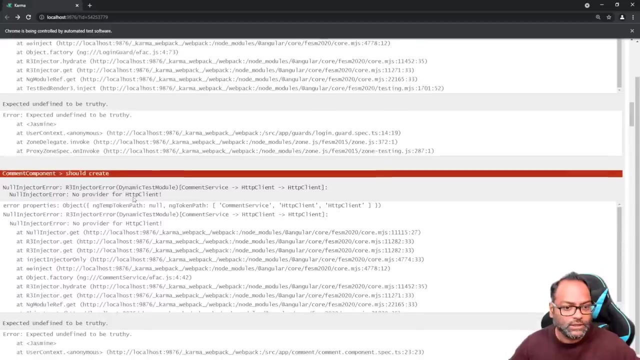 i want to use the testing model, not the original one. so once this is done, let's see, let's refresh. so now we will see, uh, less number of errors here. so it says: uh, now let's talk. let's see sdp error. so if the label coat has an error, anything, let's say rtp error is gone right, so we don't have sdp. 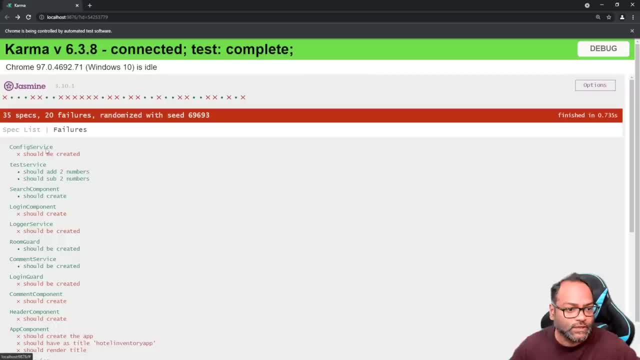 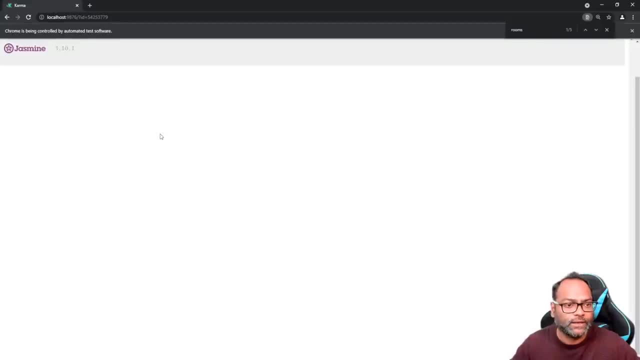 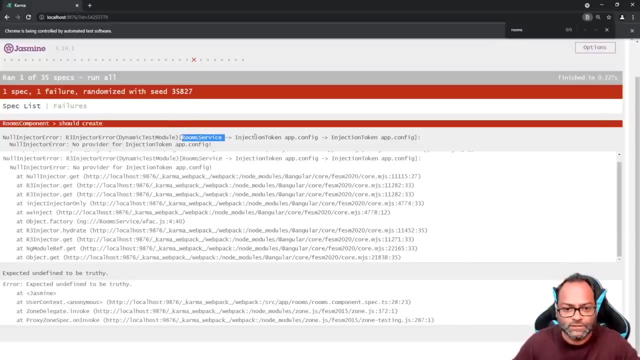 error anymore. then it says, okay, uh, this one come comment component. we don't need this. so let's go to the spec list, look for rooms component and let's go to shoot create and see the errors. so now the problem is it says room service which uses injection token. so we have to provide the 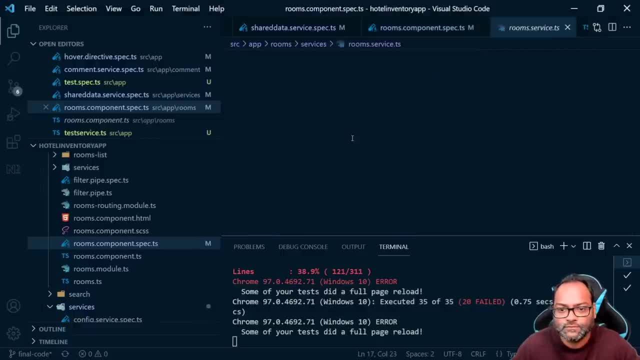 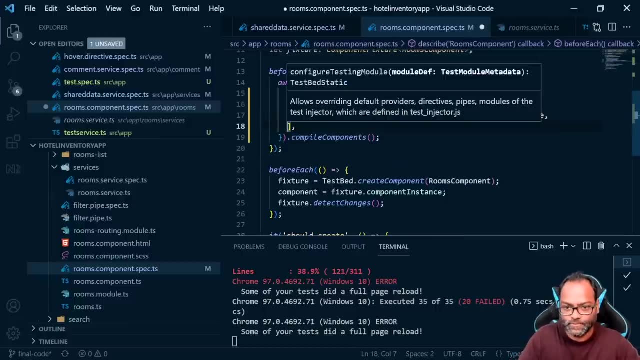 injection token. now let's see how we can do that. so now let's see how to do that rooms service. and this is the injection token which is being used so we can actually mock this. we can do something like this here. you can say: okay, provide app service config. 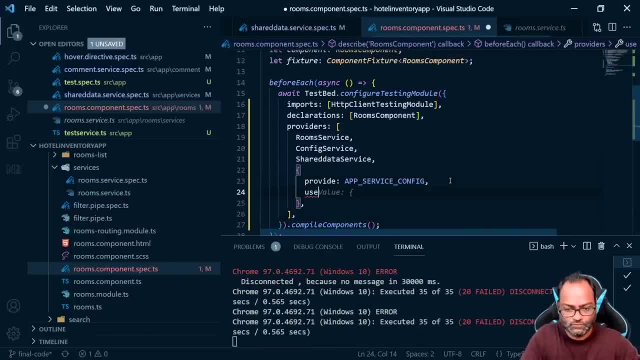 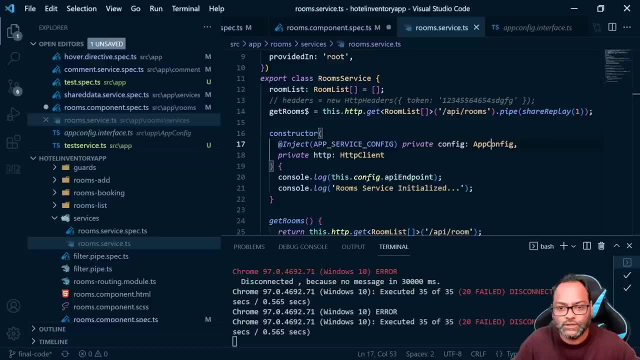 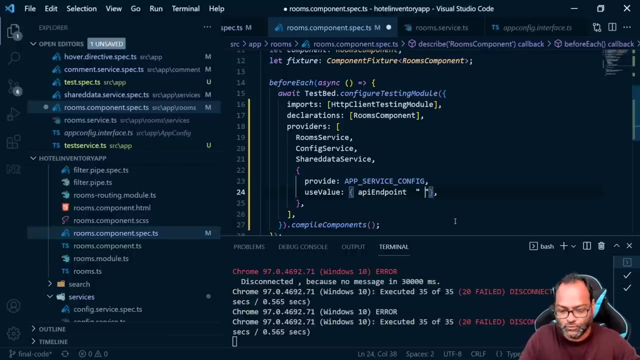 and then you can, we can say, use a value. so let's see what this app config is. so it has api endpoint. so we can go back to our componentspects and say, okay, this is api endpoint. is, this is dummy value. so you can provide any dummy value you want. and now let's see. 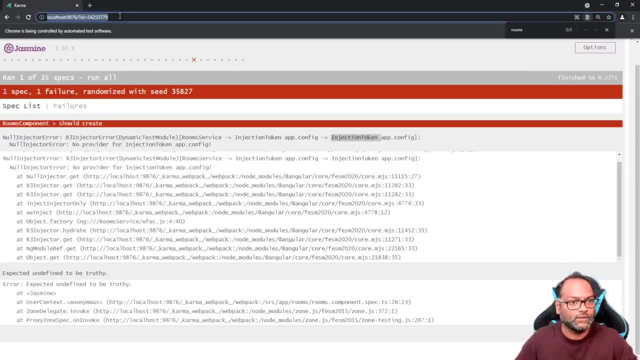 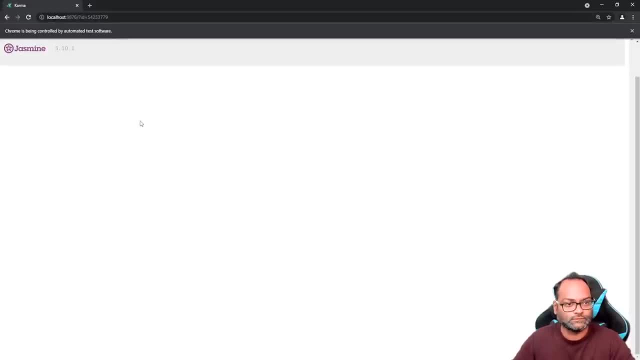 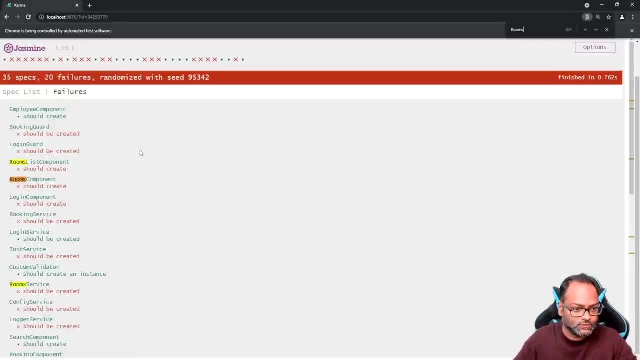 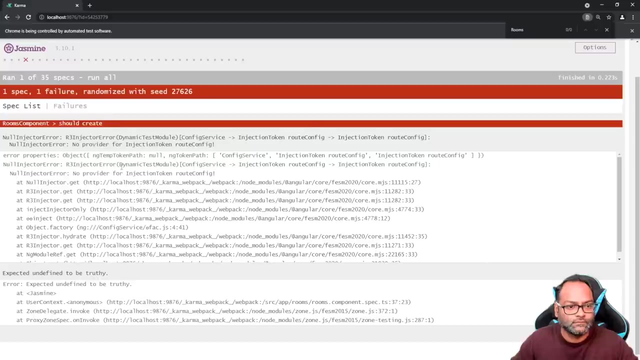 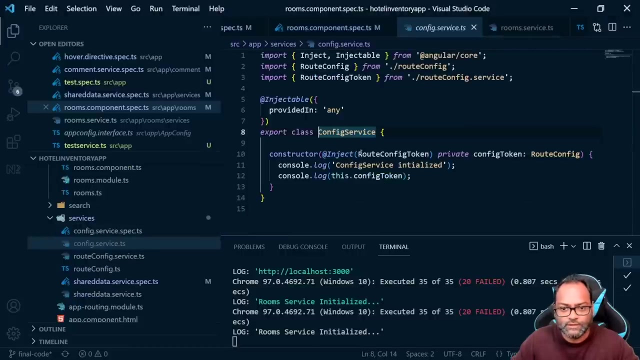 okay, chips getting disconnected. let's rerun and let's go to spec list. tomes component should create and let's see the error now. so we have now. the thing is, config service also uses a injection token. so let's see so config service. it uses injection token called config token. let's provide the service. so let's see the service. 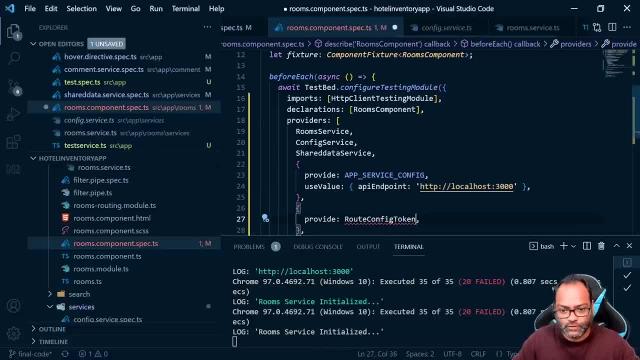 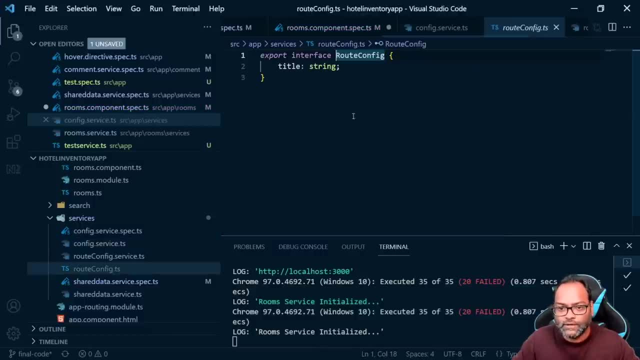 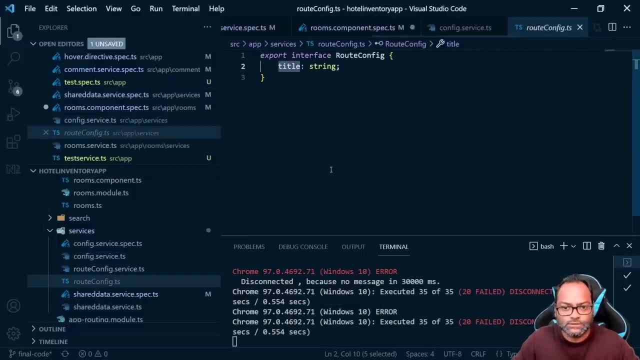 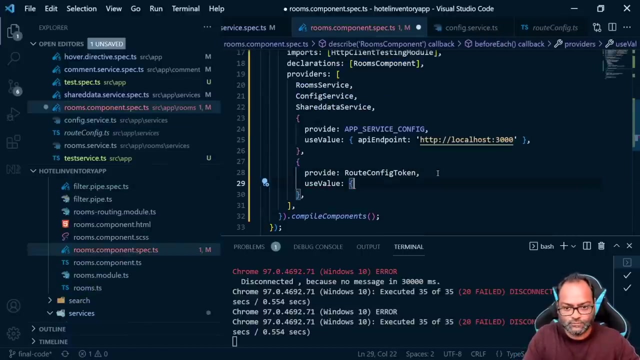 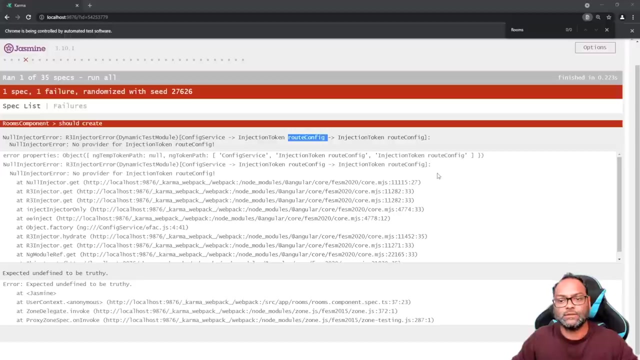 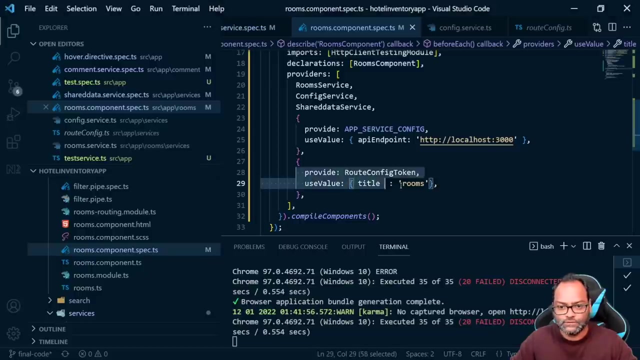 so we can say: provide cloud config token and we need the value, so write title. so here we can go back, let's and say use value, title is and let's see. so now this, this injection token should be also resolved so you can pass uh values like this. you can also re replace these services as well, so you can create an empty. 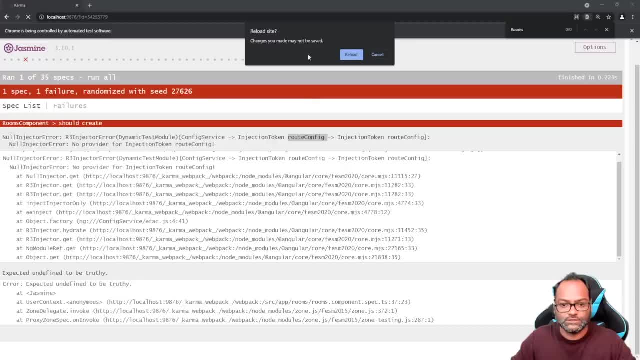 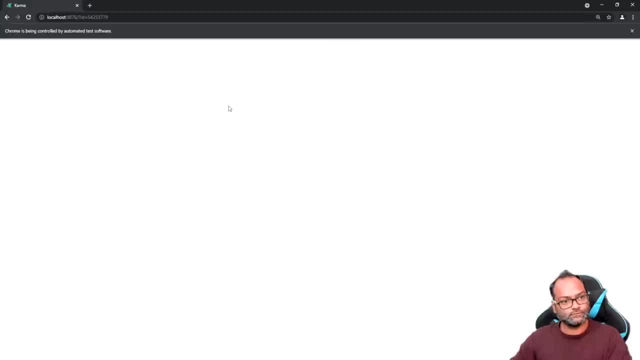 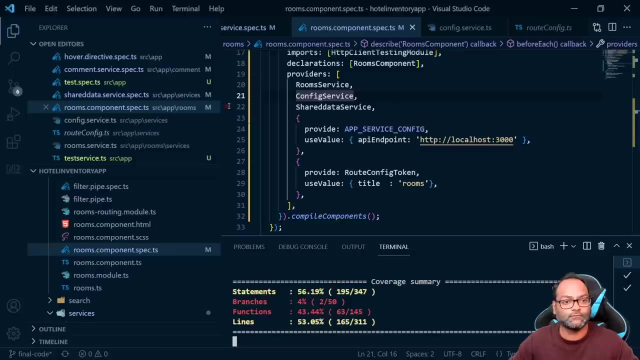 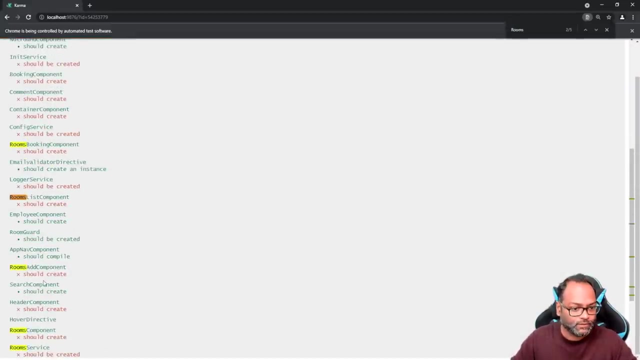 service. let me show you that example as well. let's refresh this. let's say: is it disconnected again? let's go to spec list rooms- rooms component should create and let's see the. what is the error now? so it says: uh cannot set properties of undefined. uh, undefined setting title. 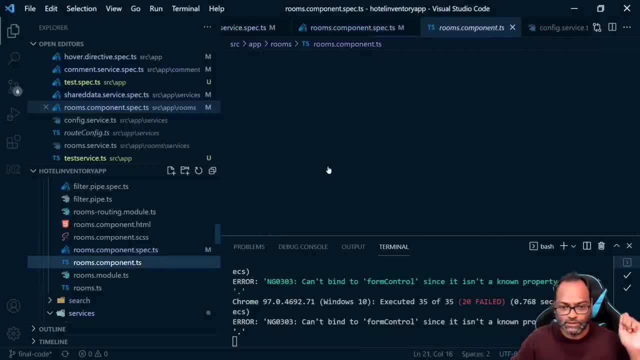 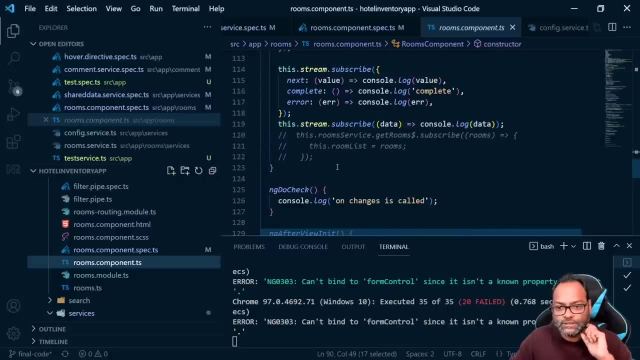 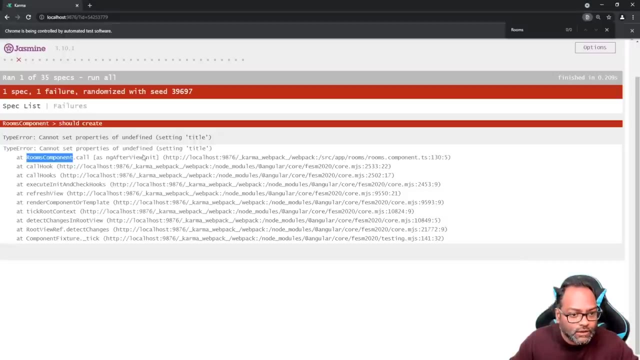 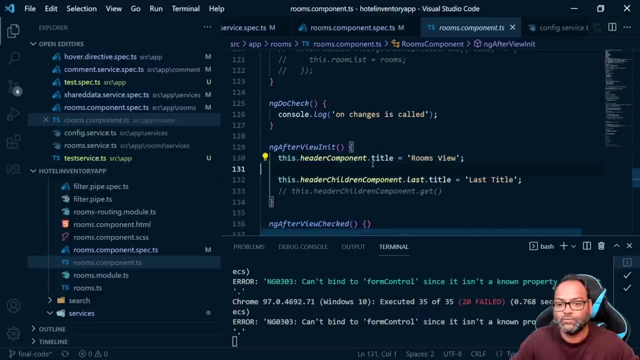 so now it is trying to call the methods which is available here. so you can see it says uh here. so these are the methods which are being called. so it is trying to now execute all those methods. so here it says uh after unit line number 130. so line number 130 is this. so it says header, component or 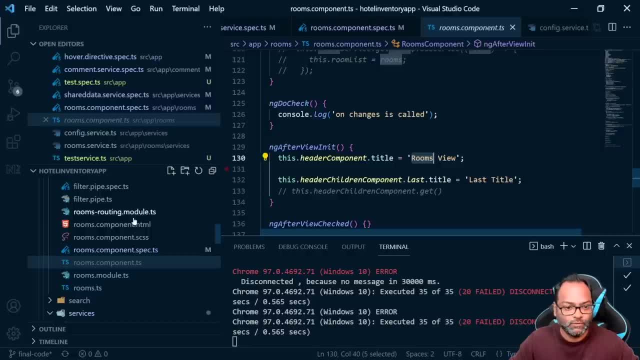 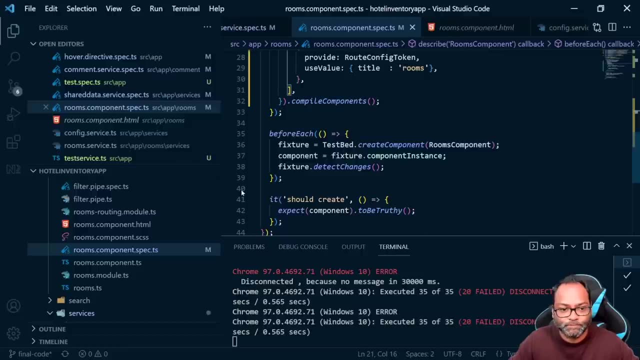 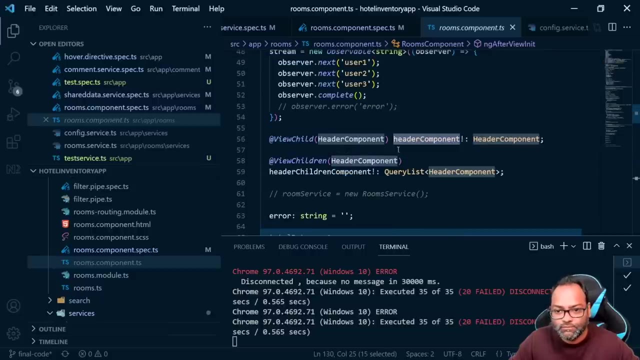 title rooms, which is a valid failure. if you remember, what we did is we have removed data component from here, so it doesn't exist anymore. so, uh, it was a valid test case. uh, valid failure, which got uh captured. so we can actually do something like this, right, so we can actually uh enable this. 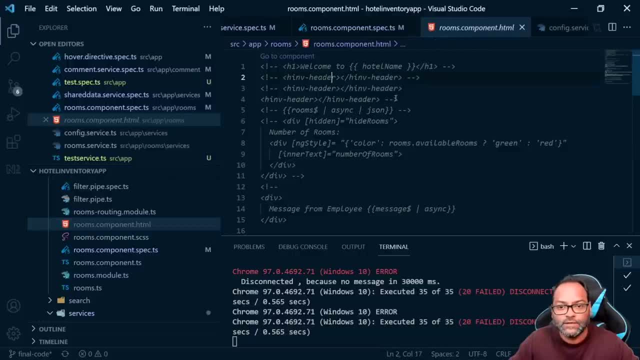 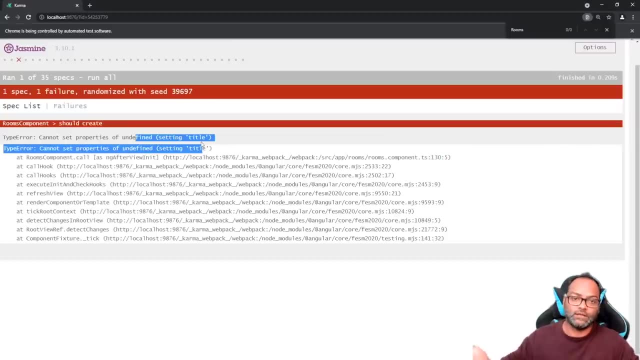 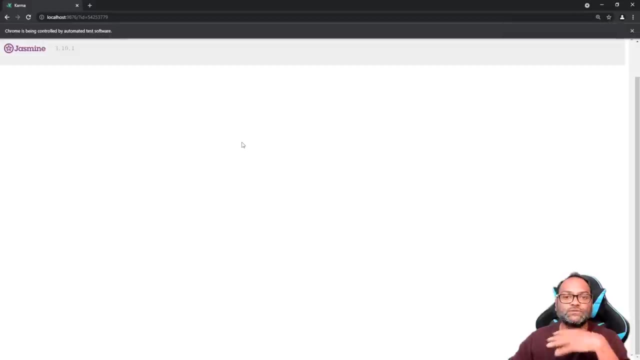 header component so we we can put one header component and see if it works right. so i can say h, i and b header and you will find not another error being replaced, uh being uh rendered. so let's refresh so as soon as you're like uh. earlier we were getting some error because the uh side of 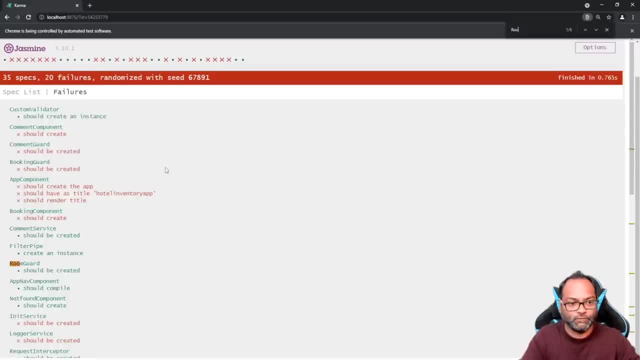 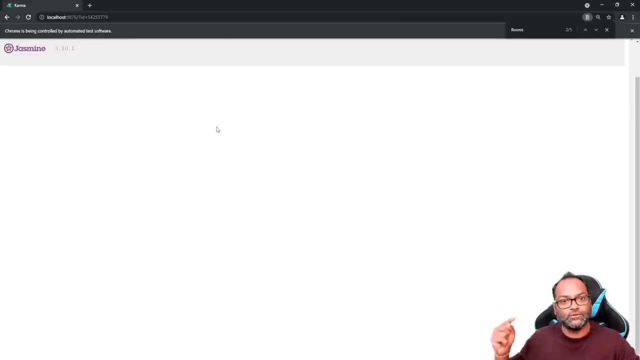 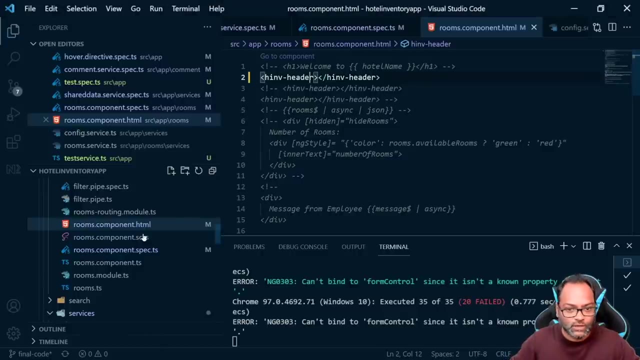 this like. this is not the way to do the uh, the way to do the uh operation. so let's just go back and uh, let's check this again. see, it is showing that all the services which we provided were not correct. so now we provided all the services, all um everything, and it is trying to execute ng on. 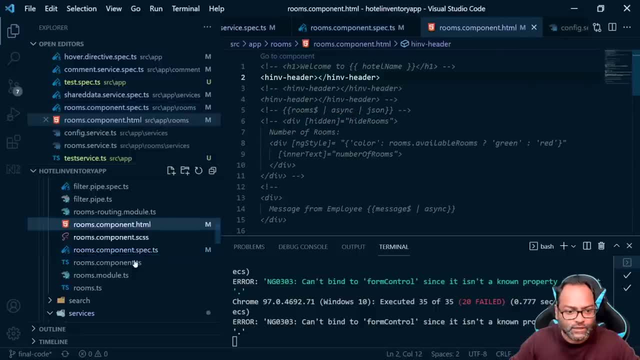 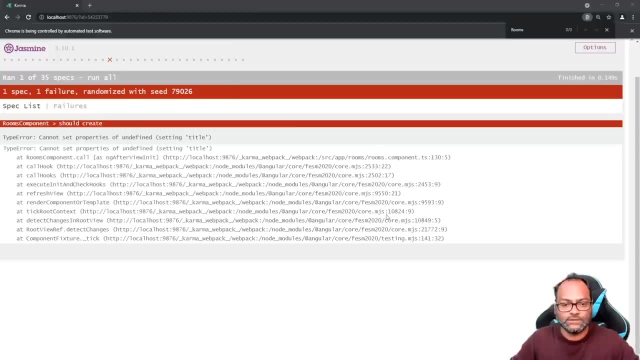 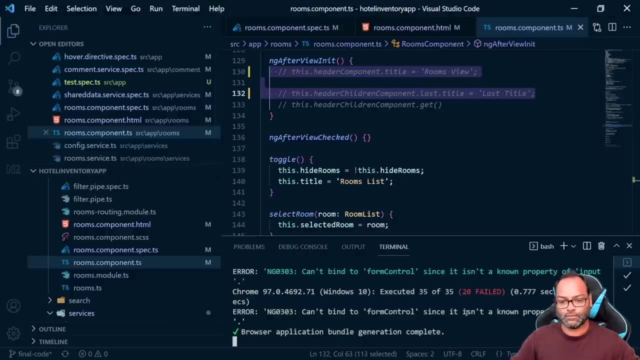 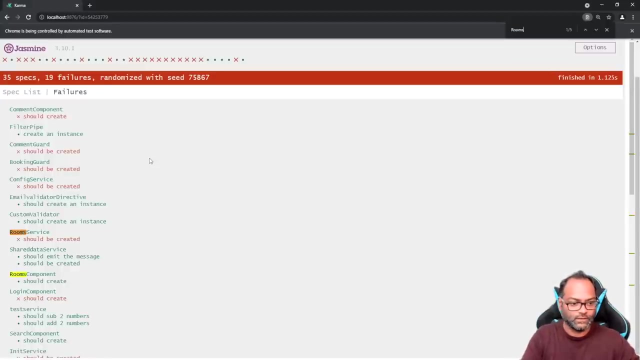 init and it is trying to execute ng after v unit, so it will start calling all the life cycle looks so. looks like there's some issue with this is: we'll save, i mean replace this and comment this out and let's see. so now we should get a different error. ah, okay, it's, it's completed, so you can see. should create. 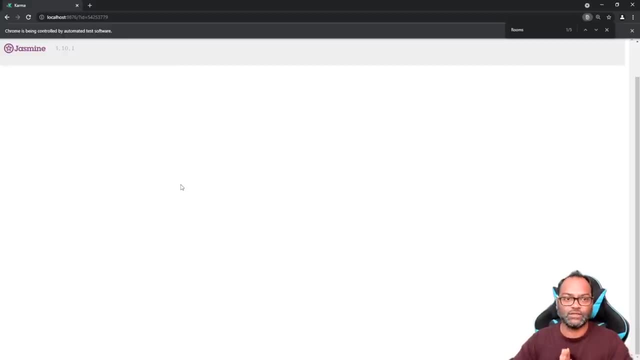 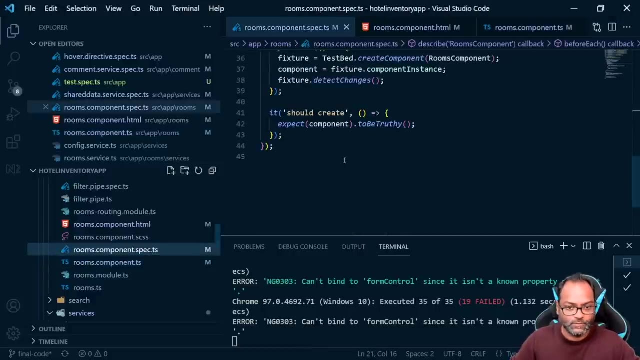 so now your component is initialized, now you can go ahead and check for the methods, right, so we can add another, let's say method, so let's, for example, let's try with toggle, so i'll say it should tangle, so so. so what we need to do is we have to. 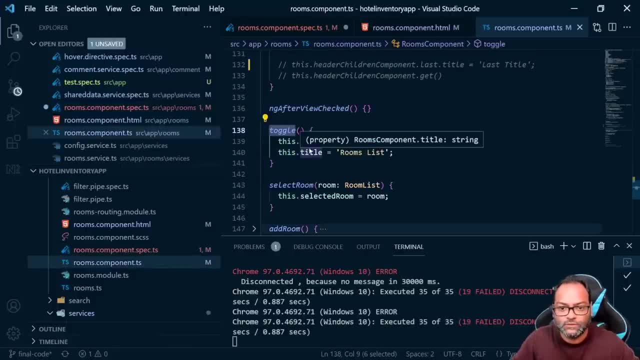 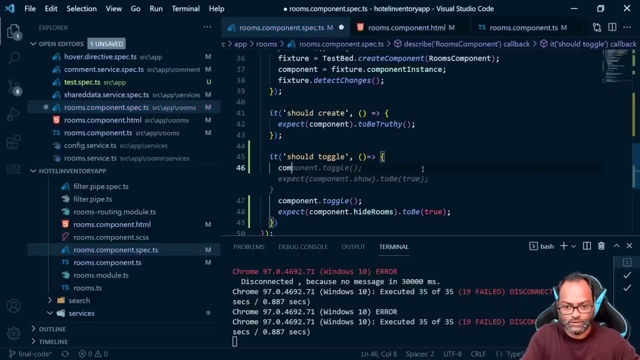 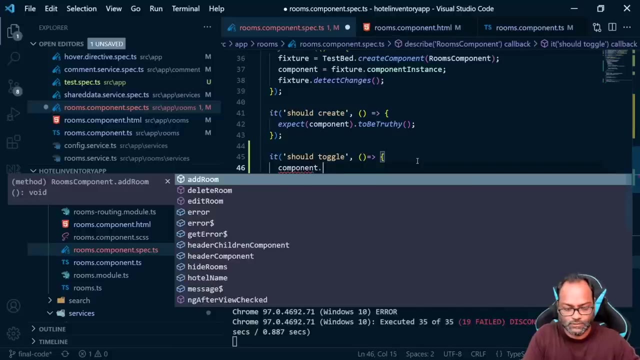 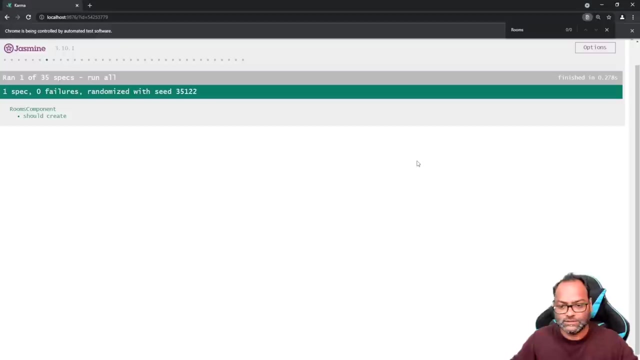 component or toggle and expect what should we expect? so we should expect hide rooms. right, so we can say: here we can set component dot. hide rooms is equals to false, and once we call toggle, we should. it should become true. that's what the expectation is. so let's go ahead and see if it works again. build the connection. 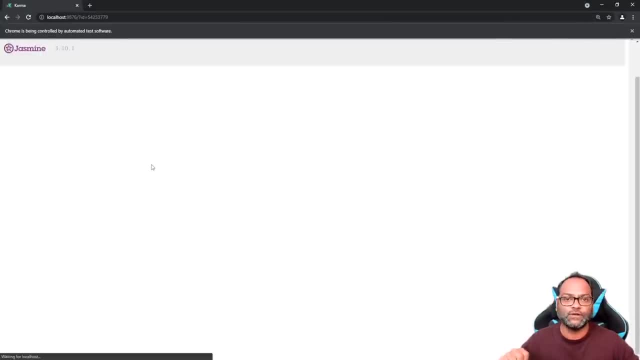 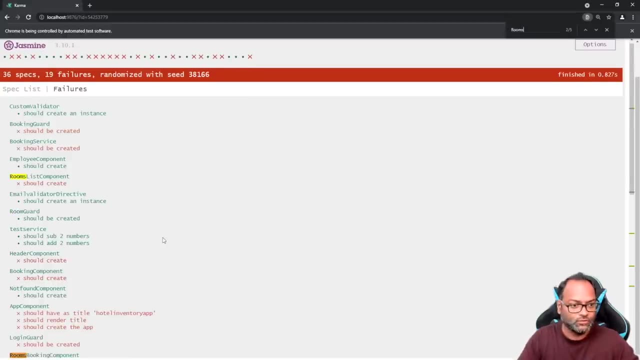 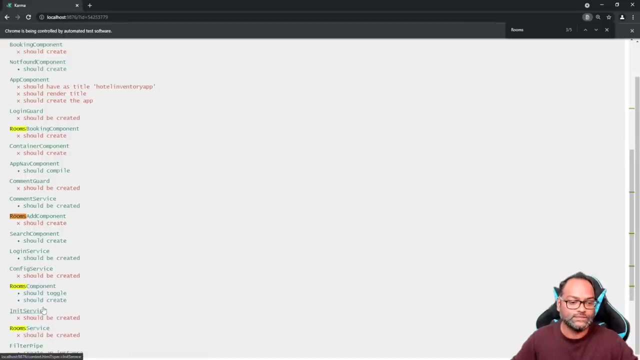 that's why people use just and or we. we can also use the reporter as your command prompt. that's also fine and let's see. so now rooms has our rooms should toggle right, so you can see: should toggle is also completed. it means now this test is also passed. so similarly you can call different methods. 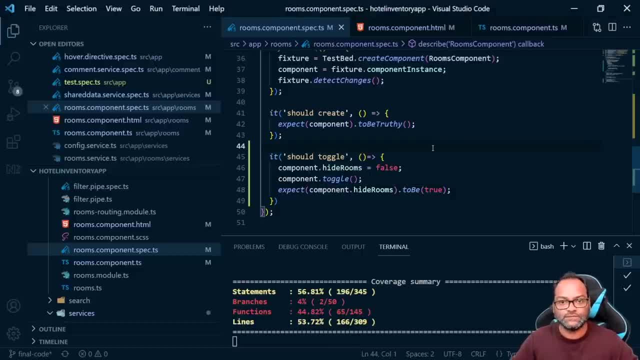 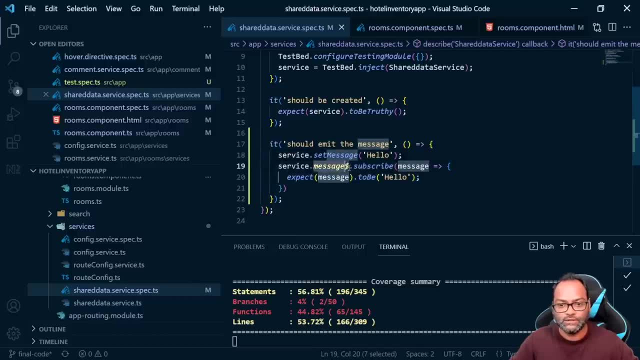 and see if they are getting completed or not. in services as well, we saw an example how we can work with observables, so you can just call the method and see if this observable is limited or not. so this is just a basic understanding of testing because, as i mentioned, testing is a huge topic. 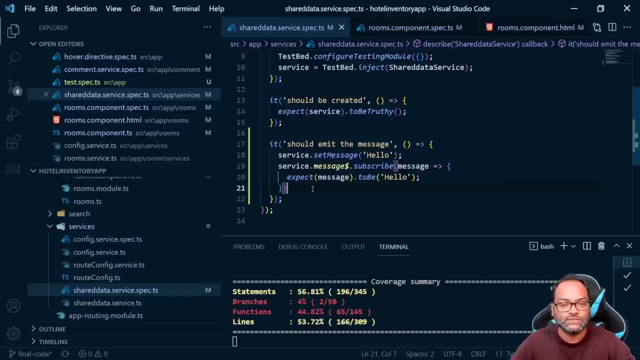 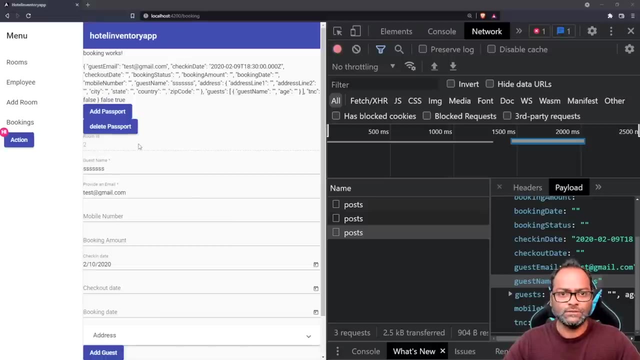 in itself and there are some courses which are- i mean we can probably go ahead and create another course covering all those scenarios. so this is it. from this particular course, this video, we will see how we can deploy our application on netlify. so there are many providers, many cloud providers, where you can actually go ahead and deploy your 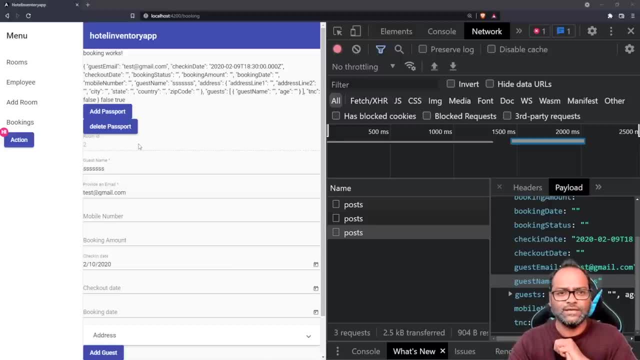 front-end application, netlify being one. let's see. it's really simple to use, so let's go ahead and see how we can do that right. so first thing which we need to do is we need to push this code on github. we have not done that. let's do it. so i'll go ahead and create an account. sorry, 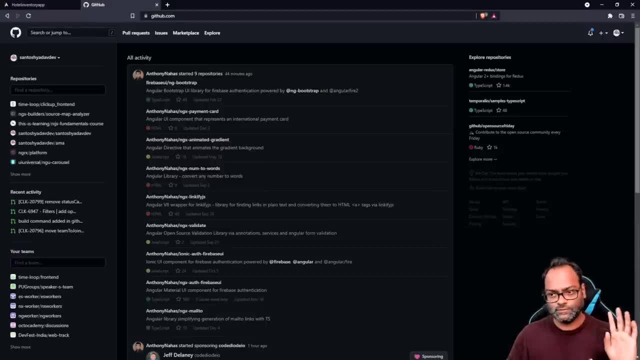 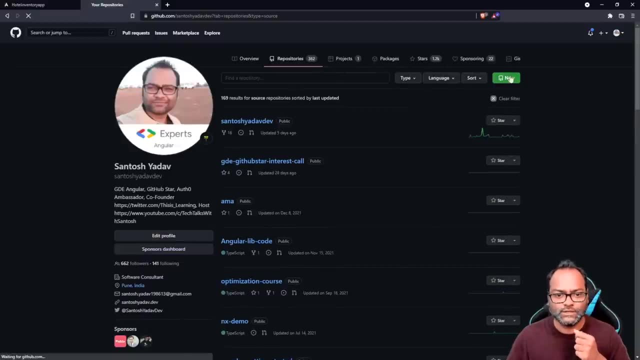 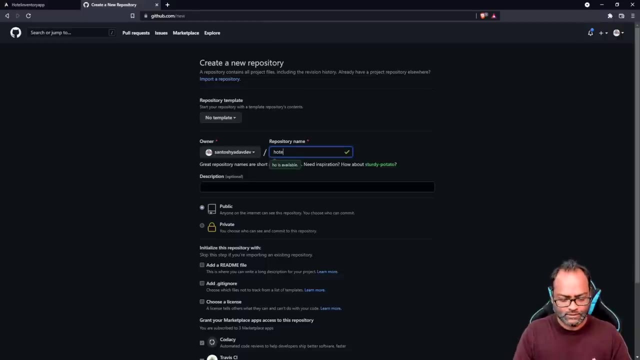 a repository. first thing which we have to do is you have to create your account. that's the, that's the step one, and now i can go to my repositories and i can create a new repository from here and here. i am going to name it as hotel in. 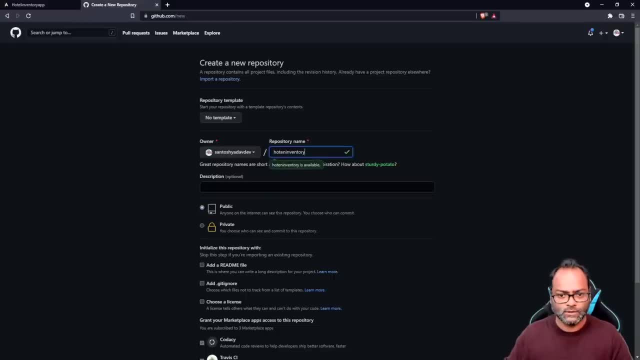 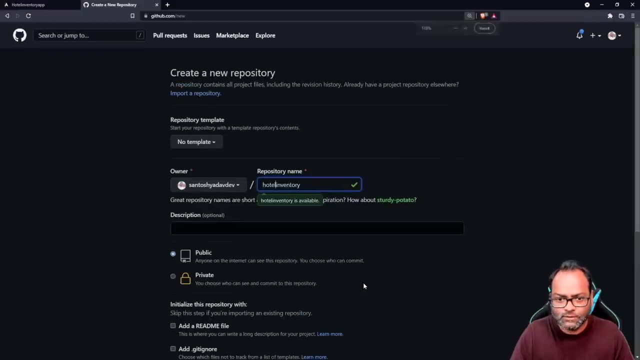 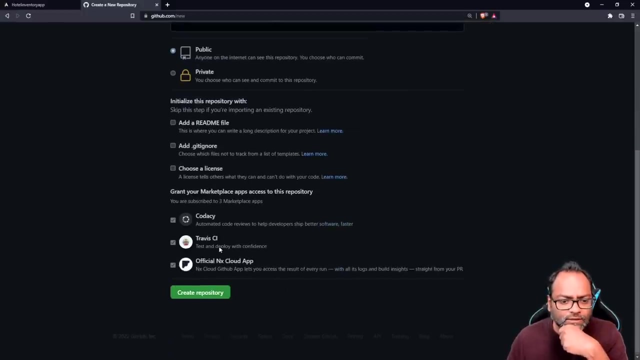 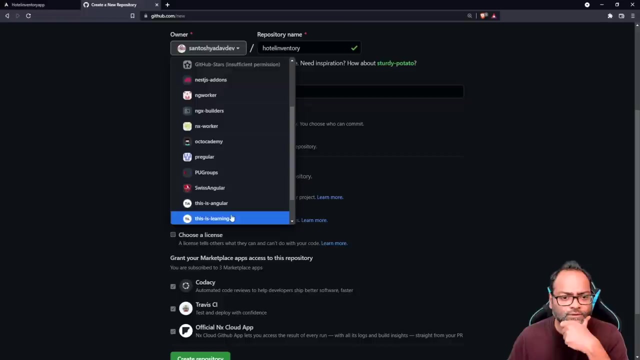 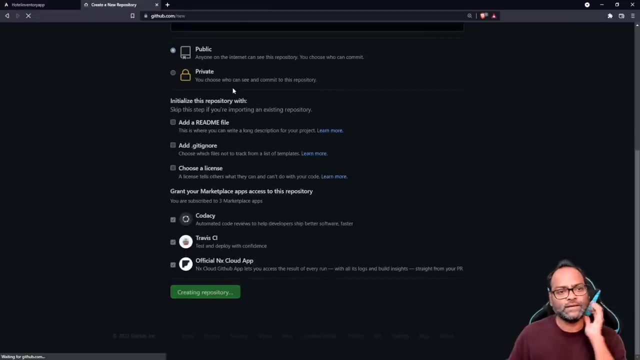 and curry. let me just zoom in. yeah, so, hotel inventory. this is the uh and let's see. i'll keep everything as as it is. let's see if we have um. right now i have made this repository public, but we'll move it to private, as netlify will. 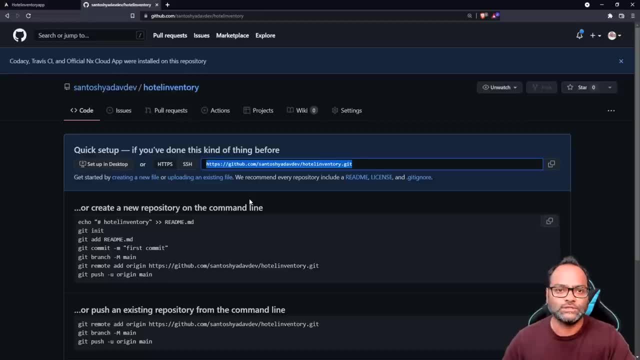 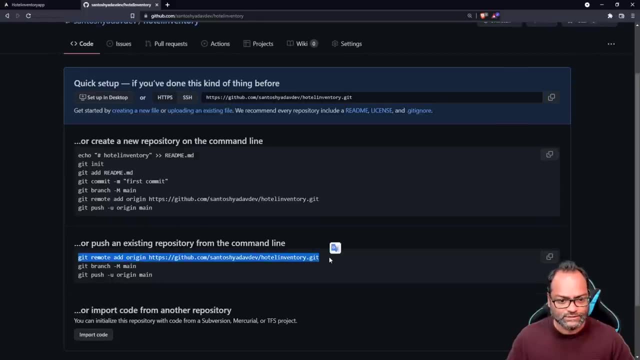 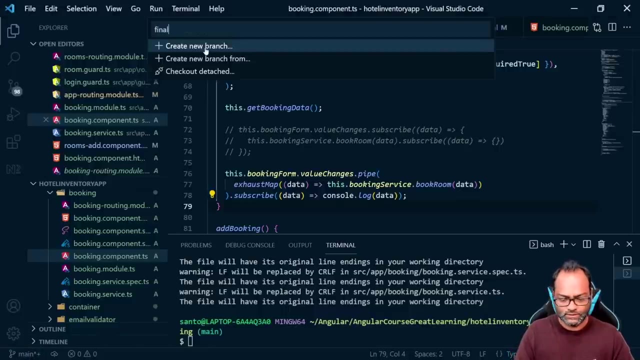 charge me for deploying and repository which is private, so i'll just use it by public right now, and once this is done, i need to actually push the existing code base, so i'll do this here. uh, get this as a branch. this is final code and i'll commit. this. changes git commit and we'll say first, let's add all. 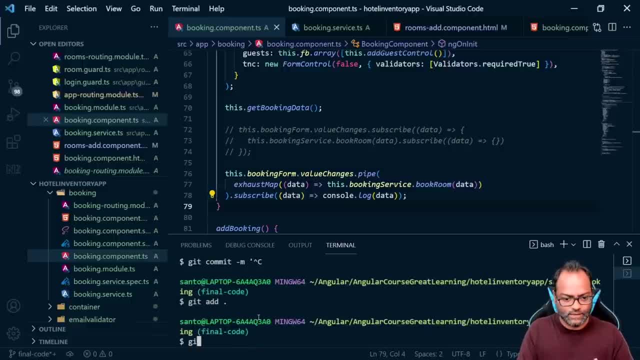 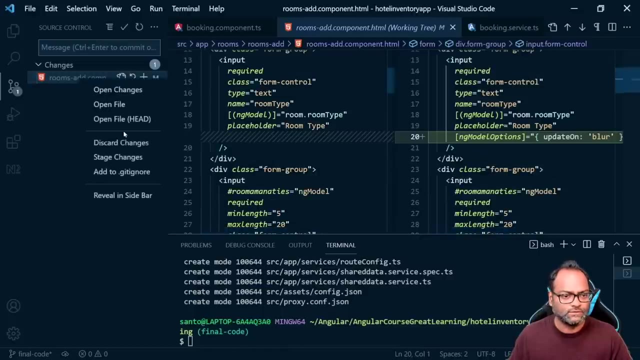 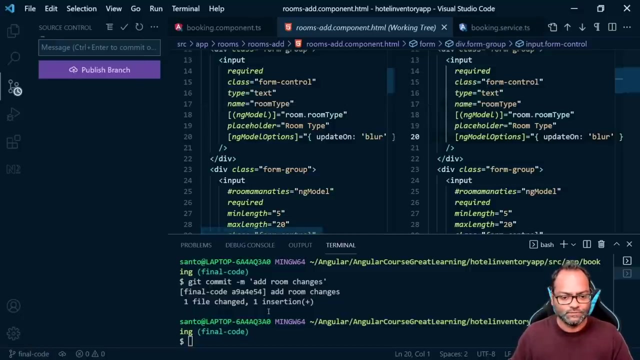 make sure that all files are added, and then we'll add a commit and we'll say: this is final code and let's move back to the master. okay, so this, somehow, this change was left. git commit: add names changes and let's move back to the main branch and as we already have the code available, so 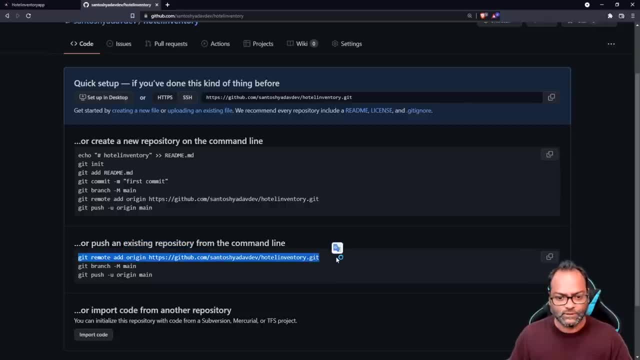 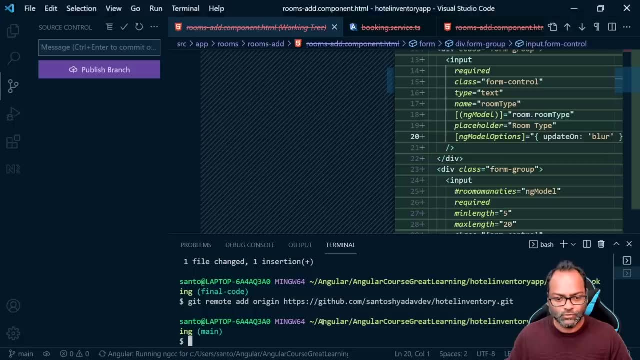 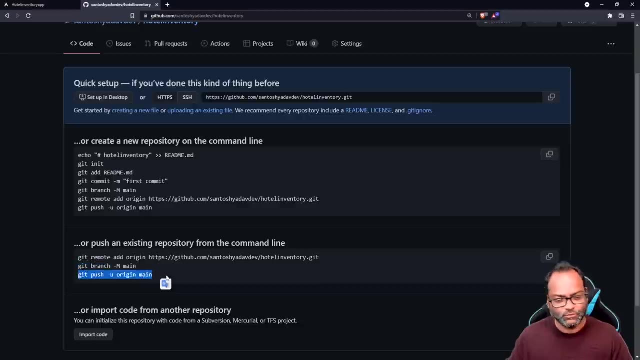 our repository available on my local machine. we'll be using this one, this command, so let's add. then we need to do is push. actually, this command was to change the branch name domain, but we already were using the branch name as main, and now let's push this code. 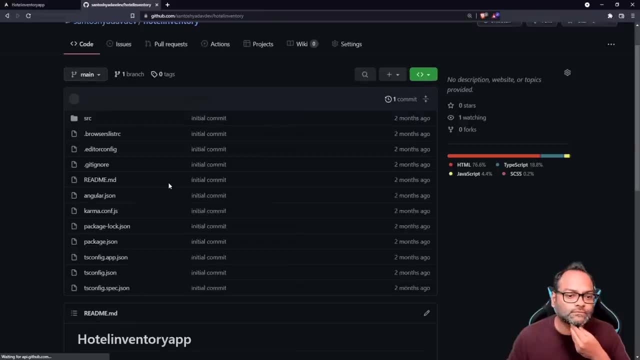 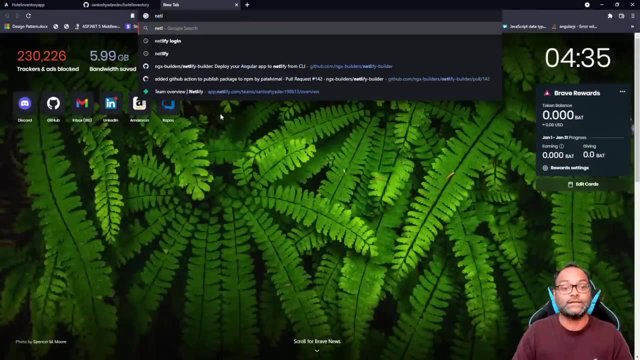 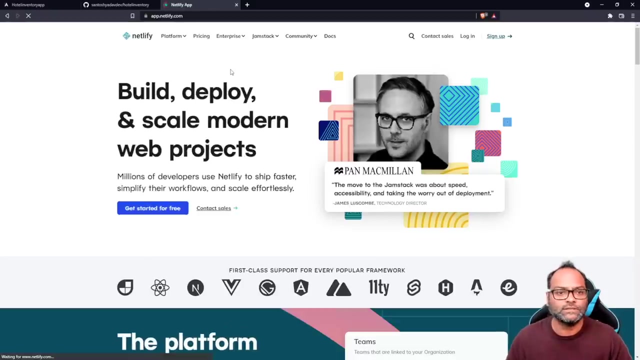 and let's refresh this and then right, so we have, uh, this, this repository, available. now let's go back to netlify. sorry, let's go to netlify. netlify login. i already have my account available. in case you don't have it, just go ahead and create one, so i'll just log in. 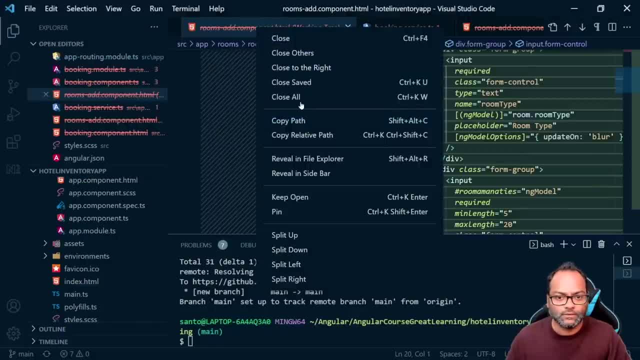 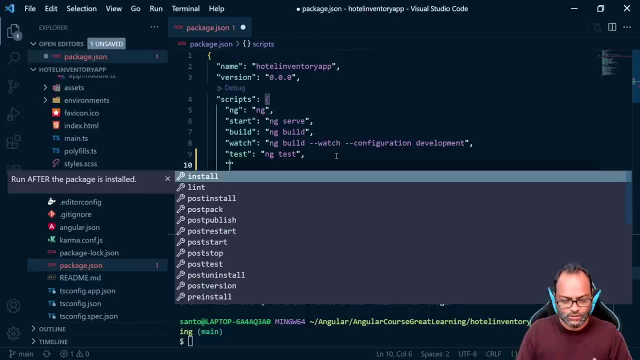 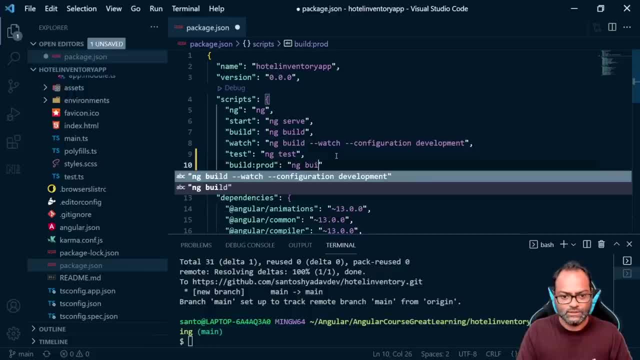 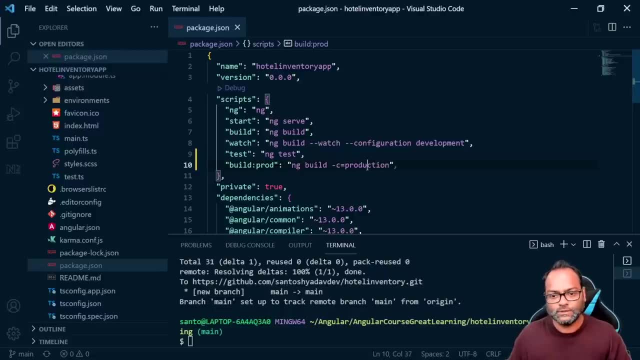 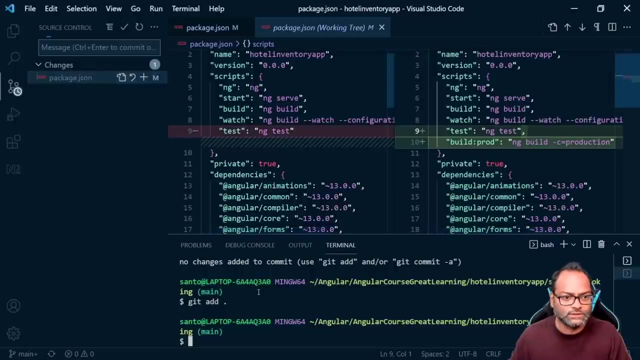 prod bundle. we have already seen the command, so we we use ng build. hyphen c is equals to production, so this will this command will be used, so i'll just add get, add git commit icon name and add prod build. okay, somehow this file was not stays properly. 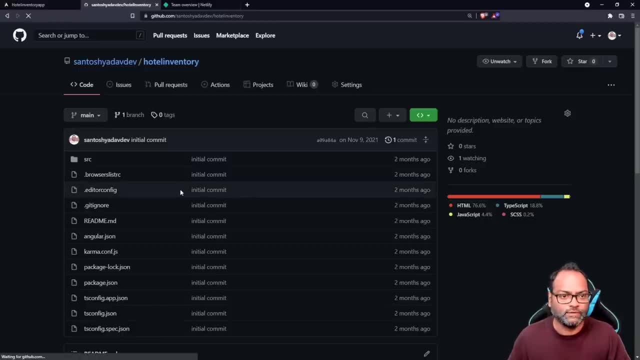 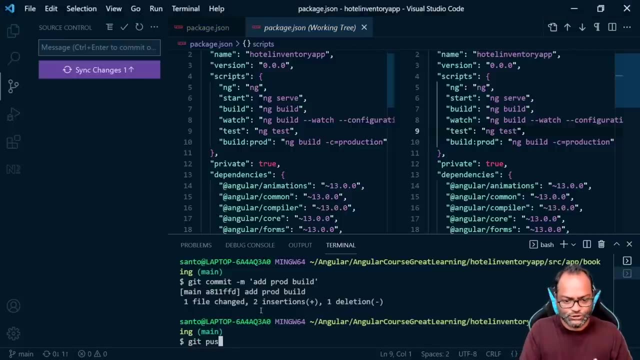 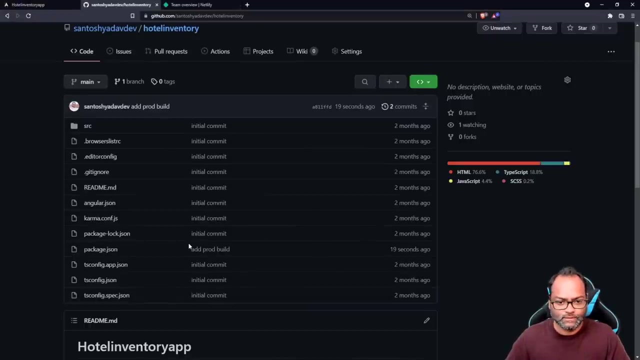 okay, so let's see if latest changes are available. and this: okay, i have to push. okay, so i pushed. i have pushed all the changes here and now it should be available. so add prod build. the latest commit is available here. let's go to the netlify. 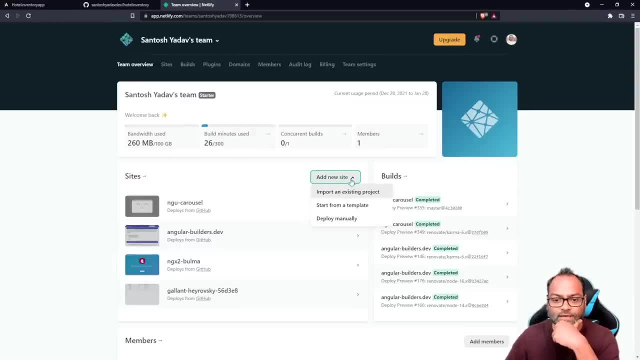 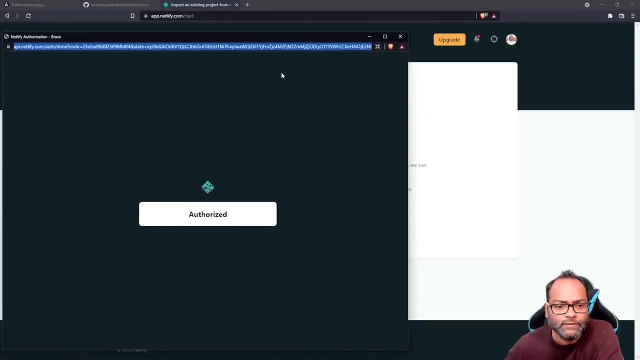 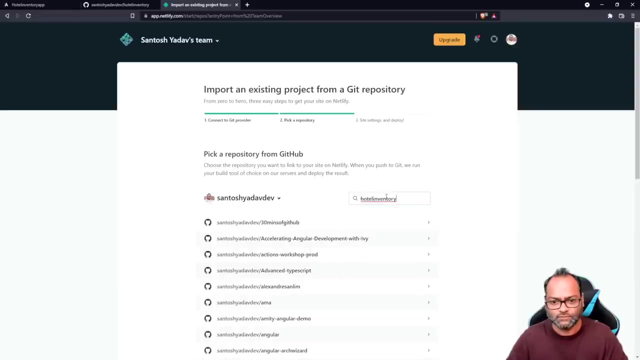 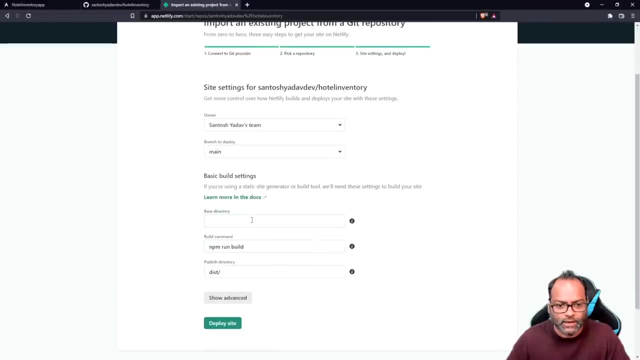 and you, we can. what we can do is we can go ahead and say: add new site, import an existing project from github, and it will uh, i'm already authorized and let's uh find this repository, portal, inventory, select, and the branch to deploy is main, okay, and uh, it says okay, if you, if you are using uh. 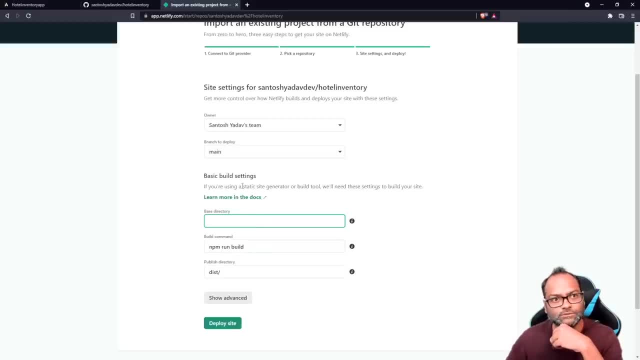 something else. i mean some. uh, if you're using monorepo, this base directory is useful. right now it's not. i mean, we are just uh having a single project. so we are just uh having a single project right now that we have we're running an mpIs. this is just a similar project. 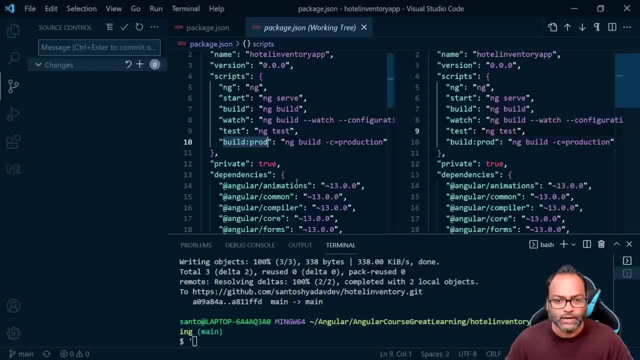 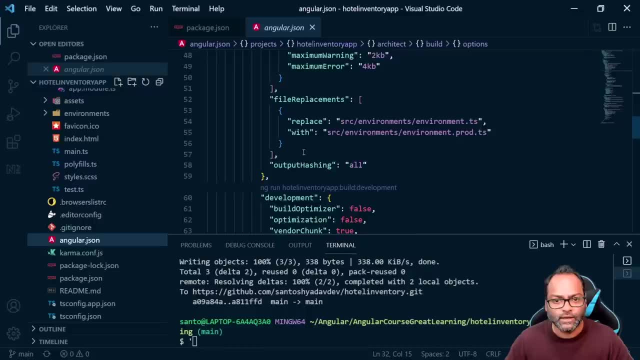 then we need to provide this plot build command here. so i'll say 1 00 0, 1 built, prod and publish directory is something which you can get from angularjson. so if you go to the production- uh sorry, build, and here configuration production, you will find 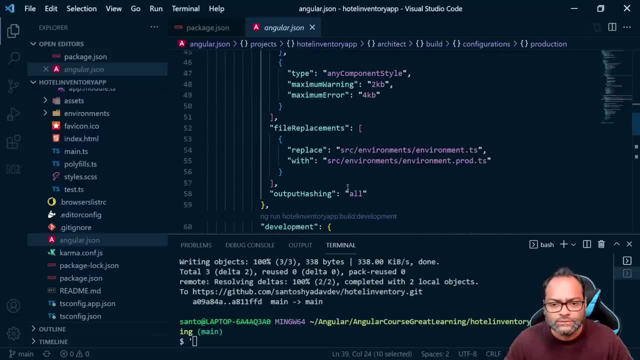 what is that? okay, so somehow it is not available here, but i will just click on publish directory transformer and run build prodbere 보� that added. here. you will find: uh, what is that? um, so i need to get theemberjson, Jason, not? so if you go to the build, you will going to get there right now. 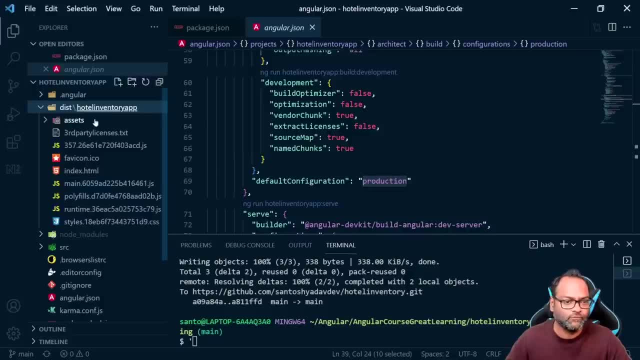 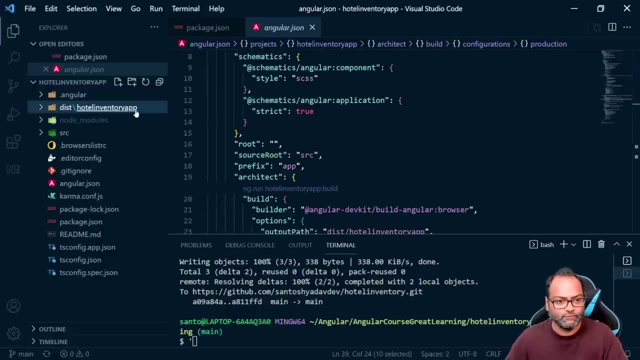 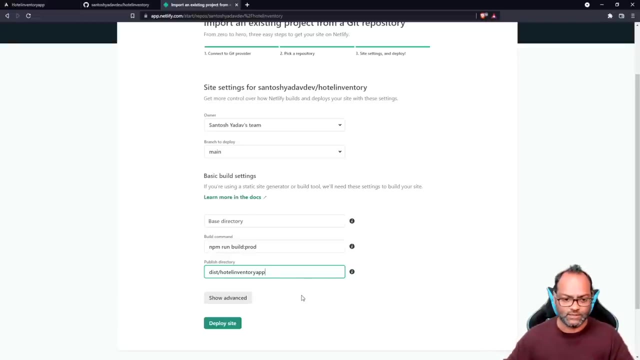 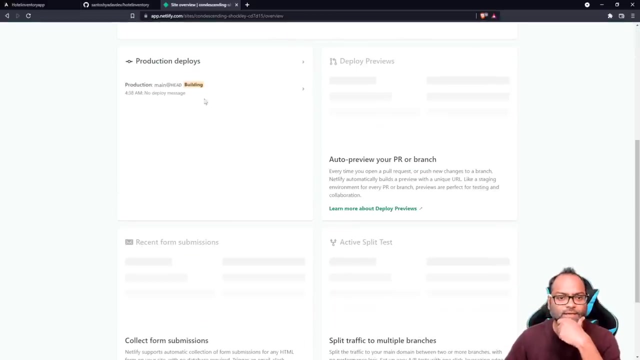 here, but generally when you create a production build, the file goes to DST slash- your application name. so this DST slash your hotel inventory am. so this is where my files will be available. so I want to publish this directory and let's click on deploy site. and now your deployment has started and let's see it. 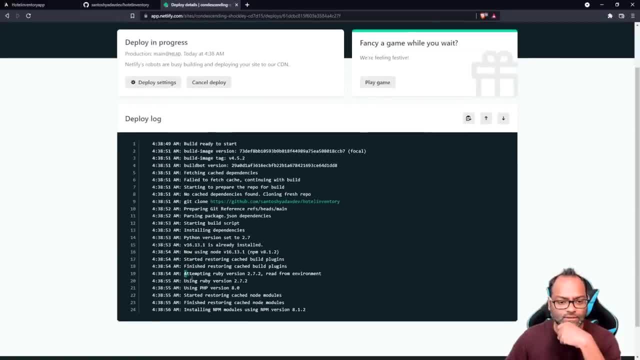 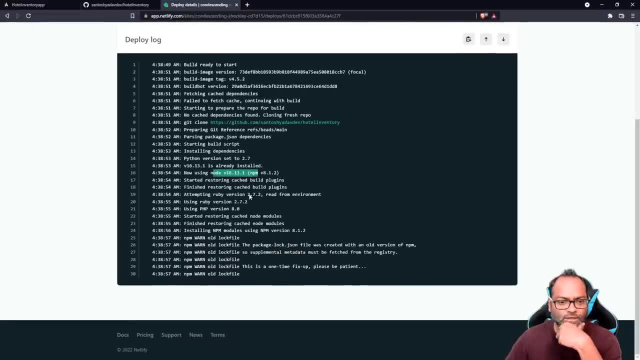 is building. you can see the log here, so it will start deploying the application. it says it is using node version 16, which is now available and somehow I already have back. I also have package log file available. I can remove this if I want to. we will remove it and 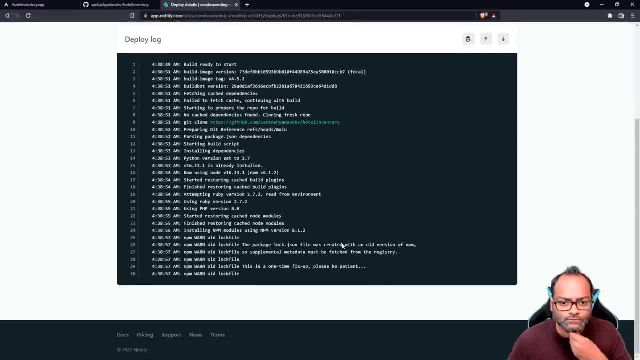 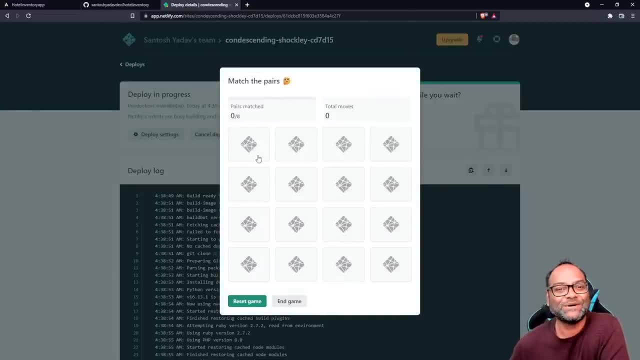 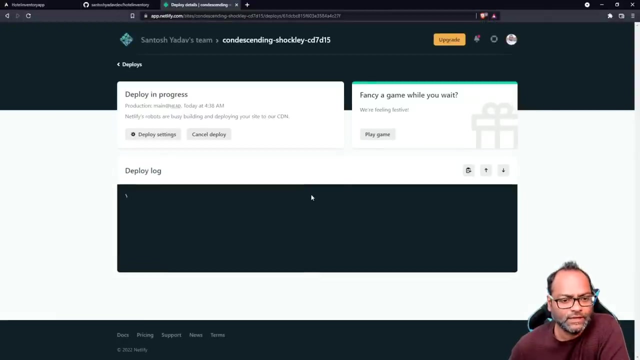 and Netlify also has this great functionality where you can actually play a game until unless your code is getting deployed right. so this is like card match: you can play. let's see, it is taking some time. if it doesn't work, we can actually do. yeah, it's done. so build command from. 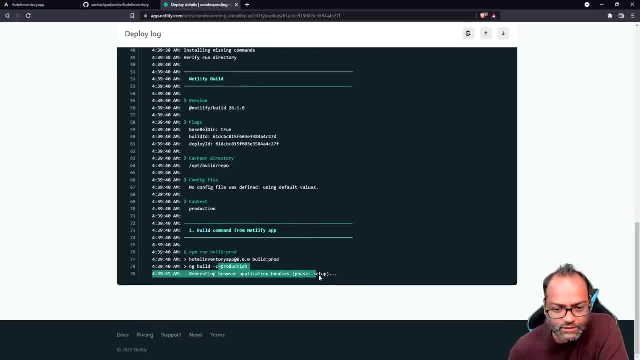 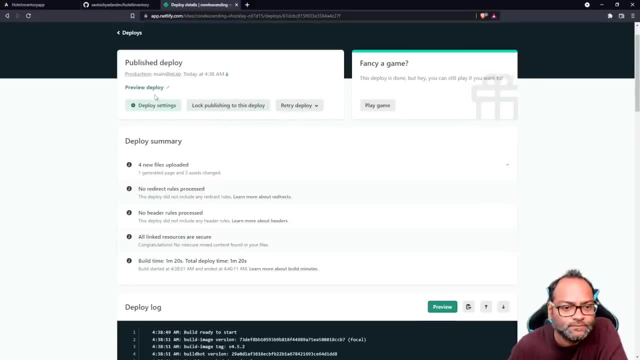 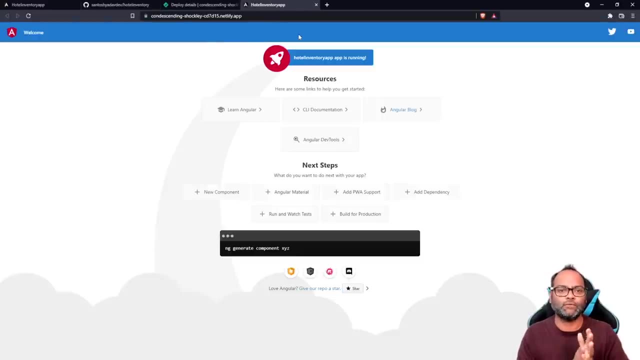 Netlify app, npm, run build prod, which it is actually generating the bundle right now, and once this is done, you will be able to see a link. okay, so it says preview deploy and you can see: uh, this is the master code, right? I mean, um, we have, we don't. 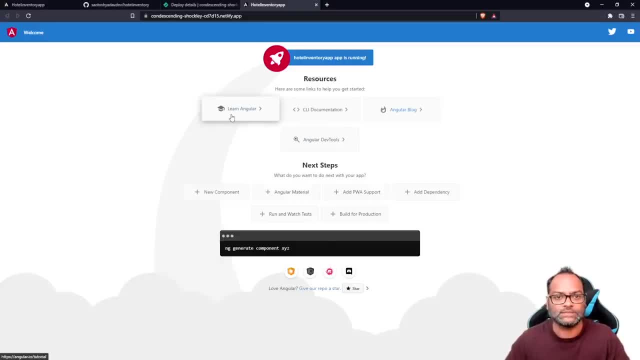 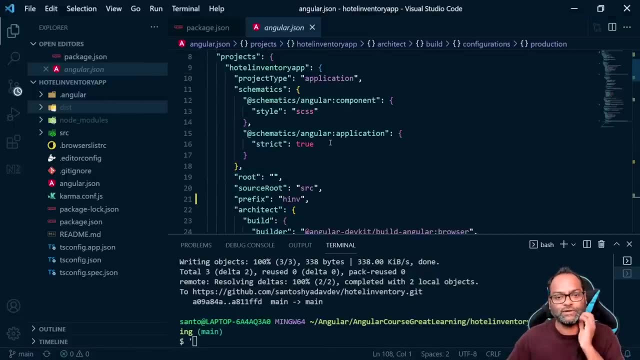 have anything available in our master code. so this is how it looks like. I mean, this is the default page which we had. so now, uh, all our changes are actually in this file, final code folder. so what we can do is we can actually raise a PR. so 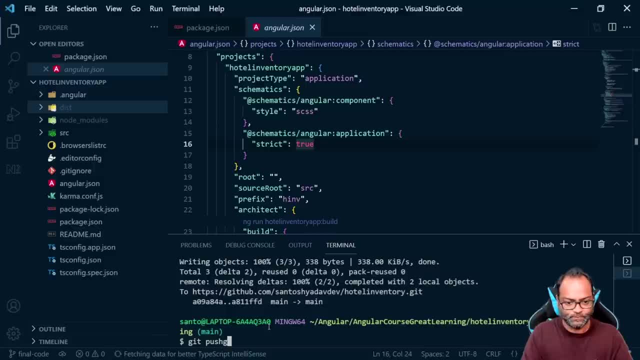 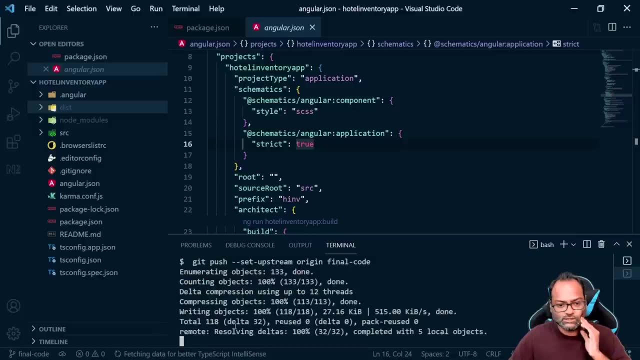 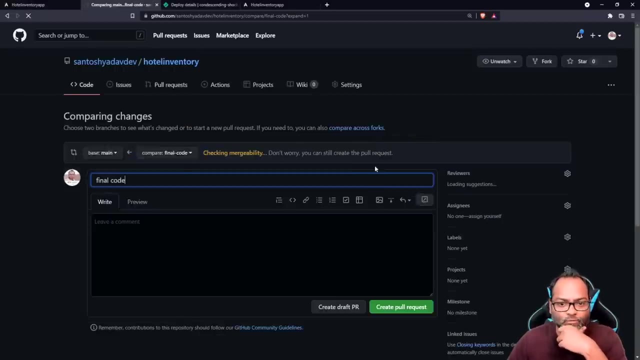 I'll just do one thing. I'll just push this branch. so you can see it says: okay, you have to push this particular branch. I mean, so I'm pushing this branch right now. let's go to the GitHub and let's raise a pull request so it goes to the final code, to the from a two main. let's create a. 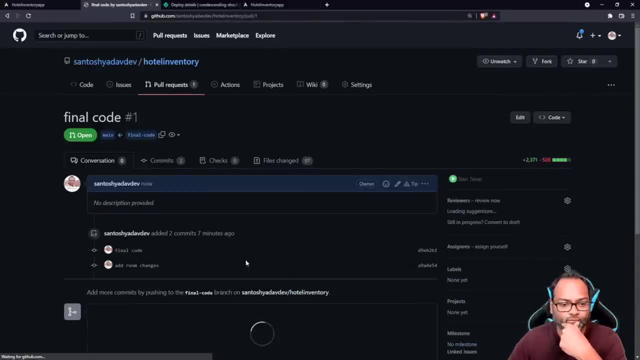 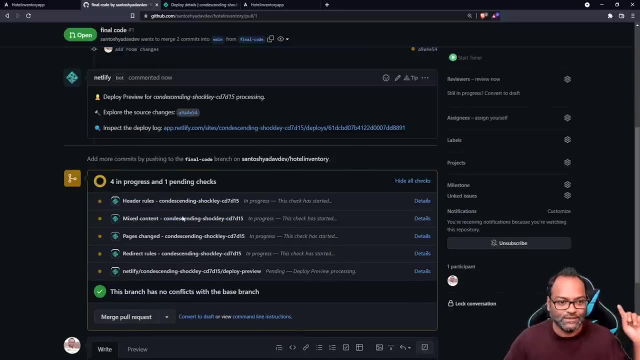 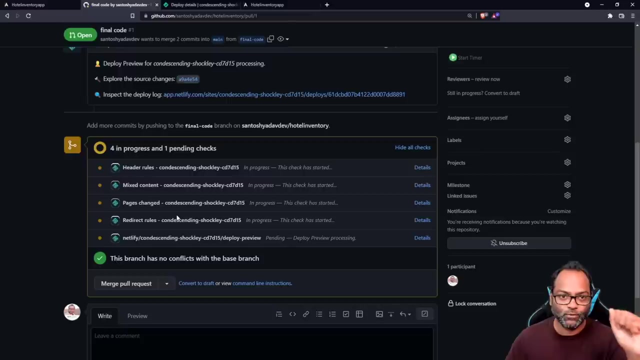 pull request and the only thing which we have to do is now it will fail. so you can see: uh, right now I we did nothing. so whenever you will raise a pull request, it will auto deploy. it will auto deploy your changes on Netlify, changes what csid means, right? so you, you should be able to do continuous integration and deployment. 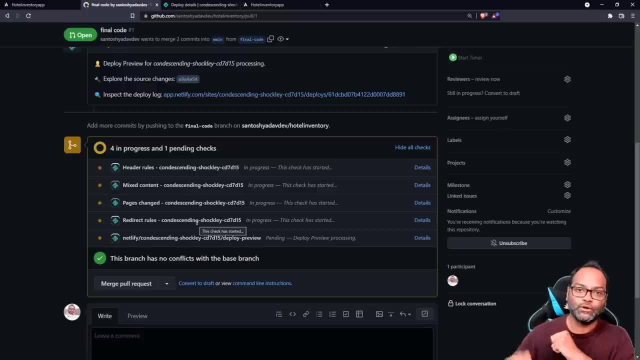 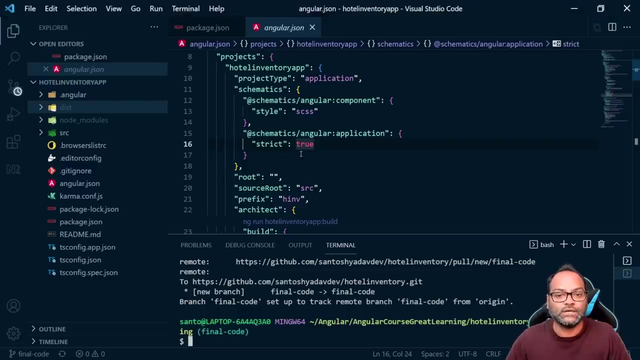 so you don't have to wait till your code is merged into the main branch to see the latest changes. here we are saying, okay, as soon as you open the pull request, it will deploy, it will merge and give you a temporary URL. so right now it is failing because we don't have the publish. sorry, build command. 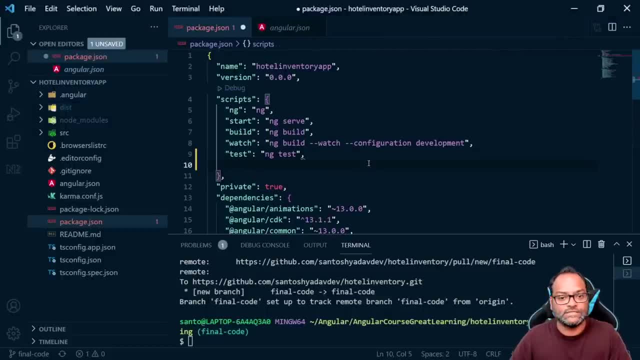 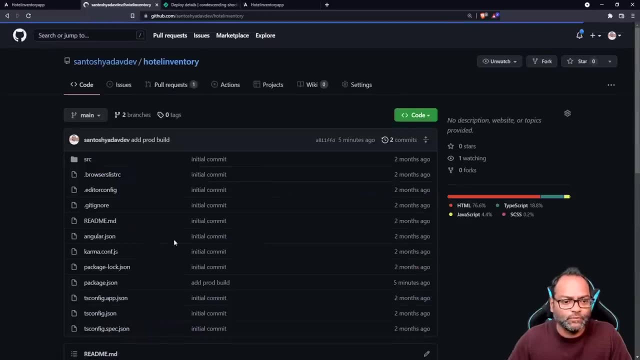 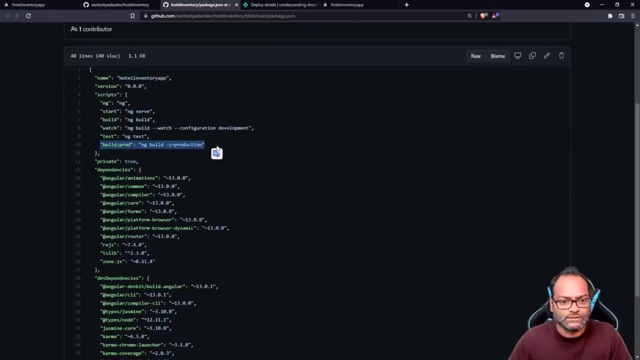 which is available here. so, if you remember, we made that change in master so we can actually go ahead and add that particular command here, and then we'll push it again to make it work and then we'll see how your temporary URL looks like. all right, so I will say this is: 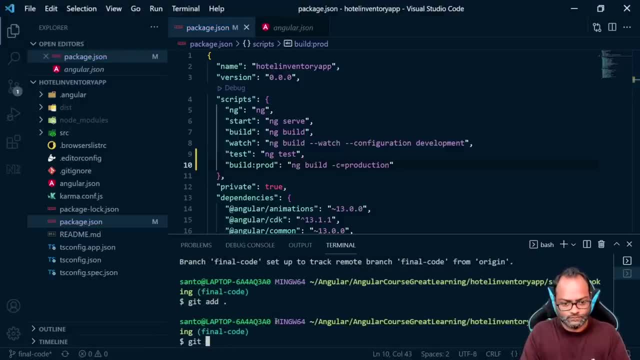 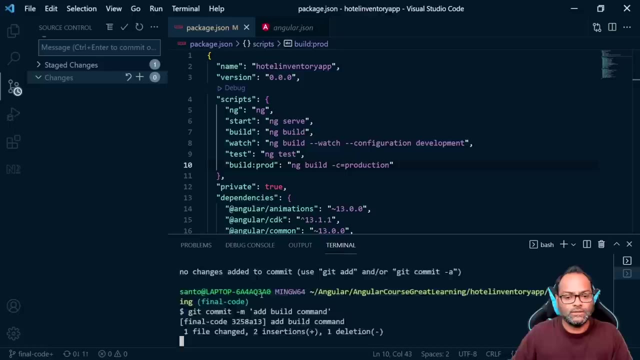 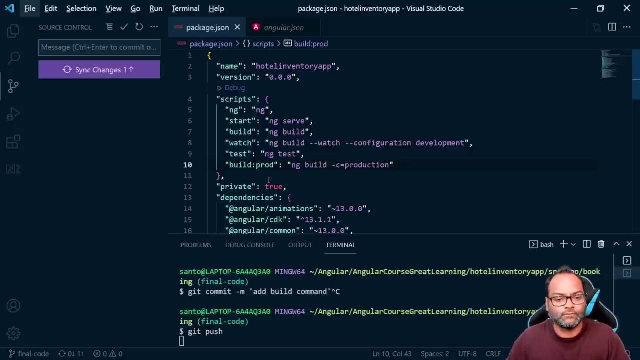 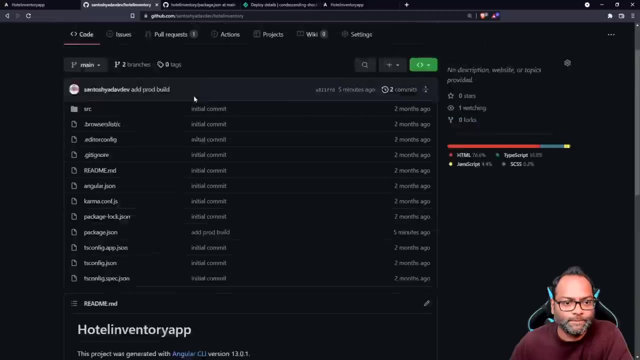 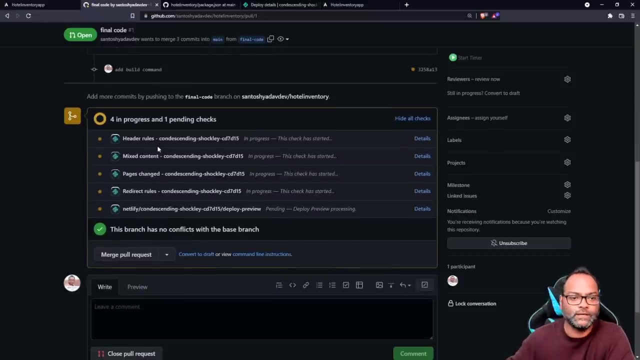 move it and add word command. okay, somehow git add is not working right now. so let's trace changes from here and let's push. and as soon as we do push, let's go back to our branch and it will try to build this code again. right, so it started the build again. and once this is done, 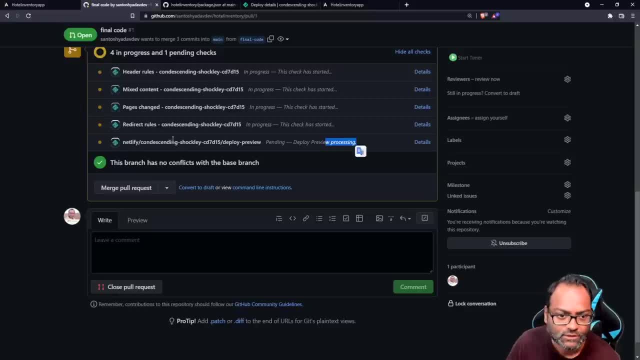 it will. you can see this is the deploy preview processing, so it will give you a link. once you click on this details link, it will open the page. it will open the application, which will be having a temporary URL. so Netlify gives a random generated URL to. 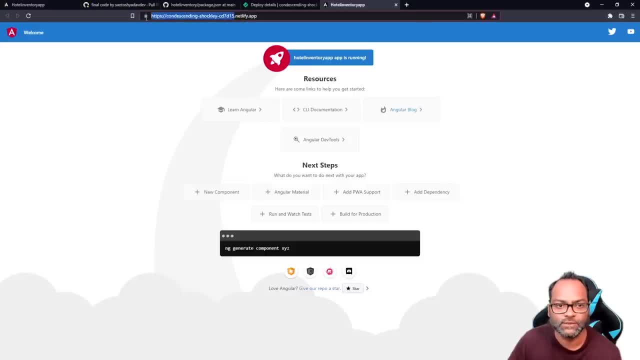 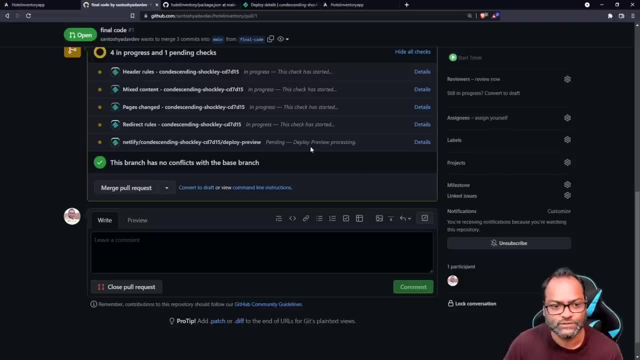 every application. so this is our random generated URL for this application, but our preview branches will have a different URL. so let's see it will take few minutes- sorry, few seconds- to complete this deployment and once done, we can see this code is available. I mean the latest changes are available here. I mean once we merge it right. so once we merge the code back to the main. 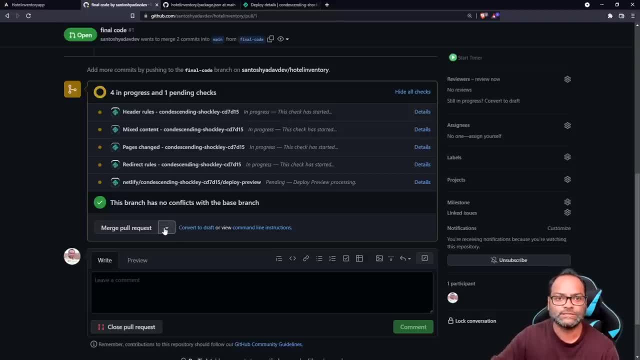 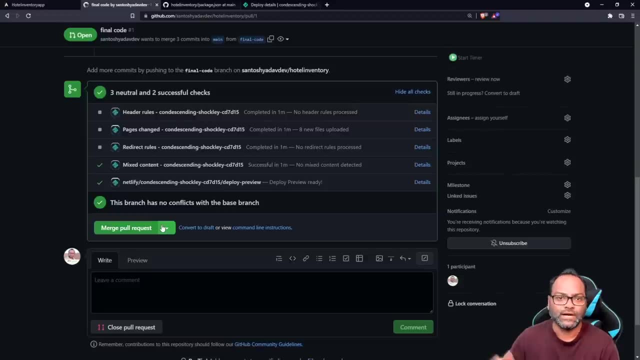 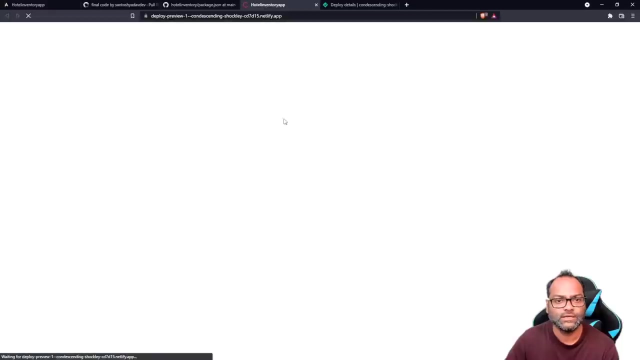 we will not merge this PR. so you can go ahead and see the difference between your master code, main code, which was just, uh, like a startup, or you can say start template using Angular CLI- and the final changes. so you can see, click on deploy URL and this is. this is the application which we created, right? 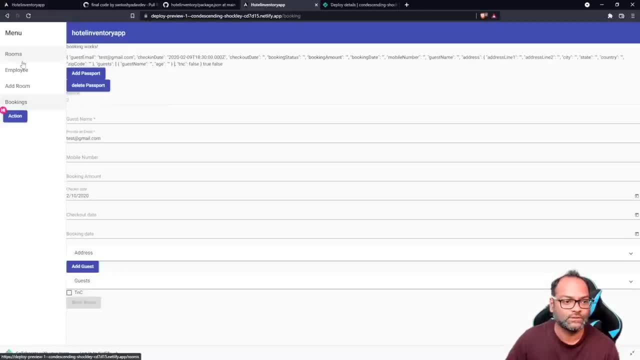 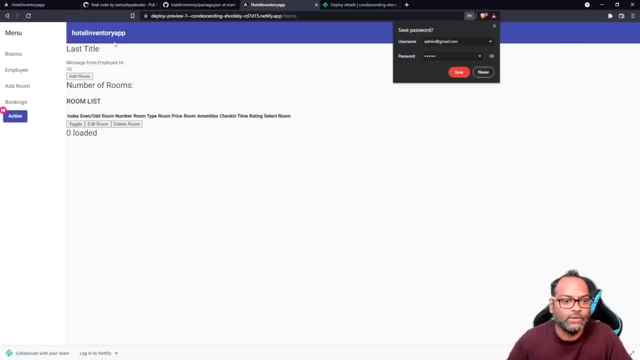 so we have this booking form available, we have this login, which was available earlier, right? so admin, and we can do admin and you can see you have your view available here. you can just click on send message, which is available here room where this message is available also, so you can say deploy preview condensing. so this is your. 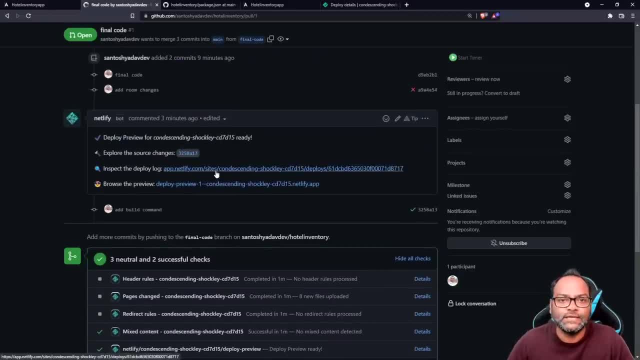 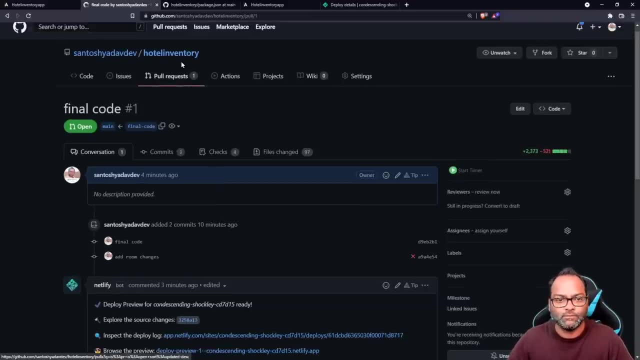 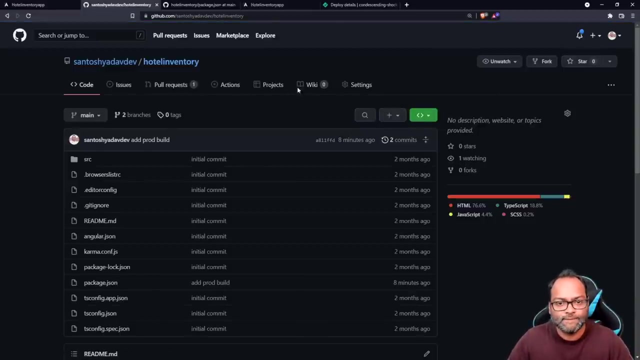 preview branch. so this is how you can actually set up your CI CD for using Netlify. go ahead and deploy your application. Netlify is free for open source. I mean, right now I'm just going to make this as private so you you can go ahead and get the access to this code later on. so 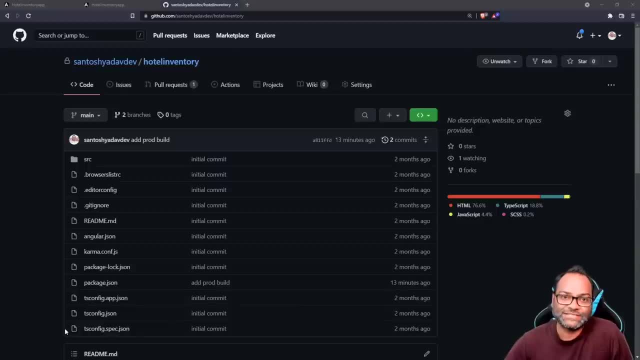 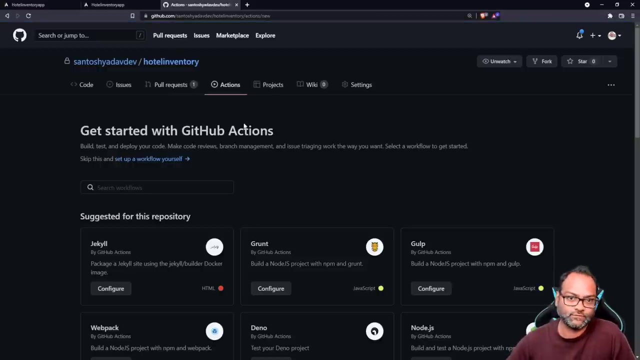 in this video we will see how you can also use, utilize GitHub action to build your application. so remember, we are just talking about building, because we have already have CI CD available with your Netlify, so GitHub actions is something which can help you to automate the stuff. so here we. what we are going to automate is, on every pull request, a new build should be or: 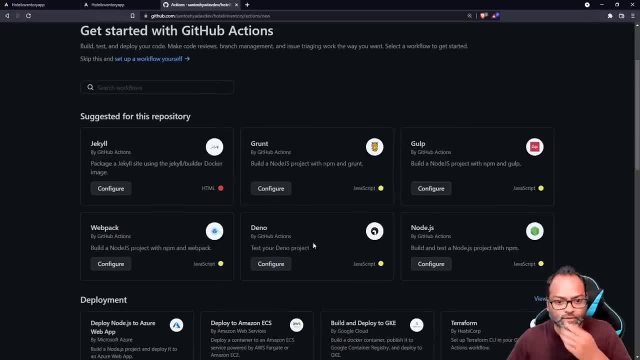 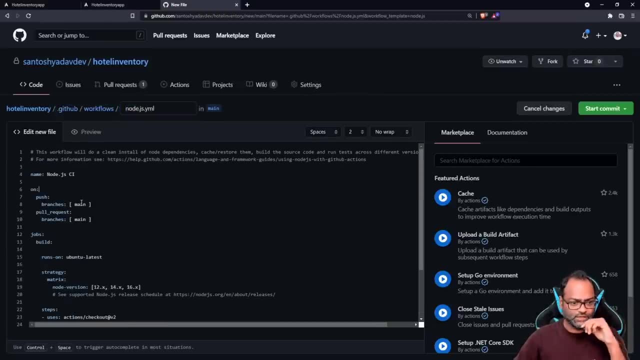 your build should be done right. so, uh, here we can just go to nodejs. we will use nodejs to build our open, a nice template. so it says, okay, which branch to uh on push to this branch, build on pull request button, build which server to use. so we are saying, okay, we will be using open to which node version. 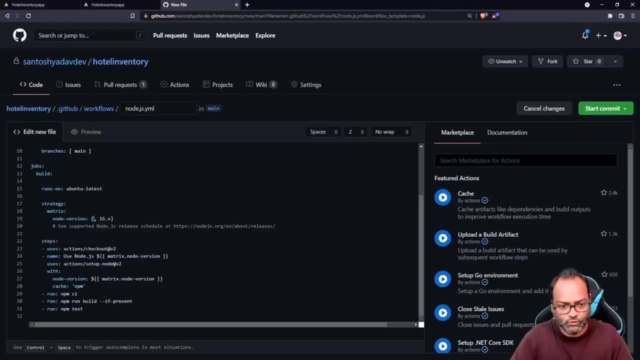 to use. we will be using only 16 because we don't want to utilize much of resources, remember, for open source net. uh, this GitHub actions is free. I, I have the pro license, so it it is. uh, it gives me 3000 minutes, if I'm not wrong, 3000 minutes worth of build time for free, And then we have 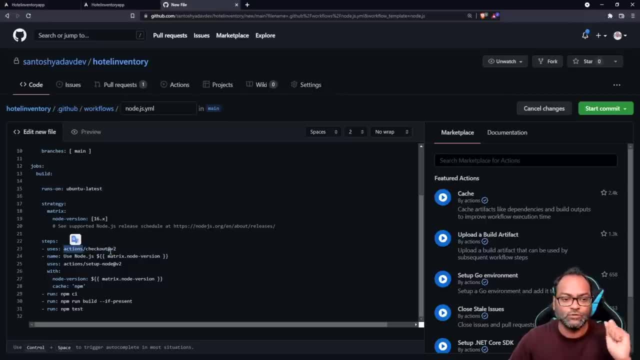 this uses. So it uses some GitHub actions to check out my code. So checkout is some term which we use in GitHub, in Git to copy the code and make our own version. So we check out this code and then we use this node version, which is 16.. And then we are caching the NPM version And 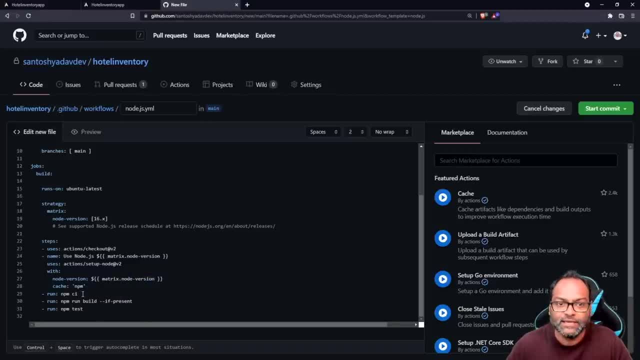 here we are running NPM CI. NPM CI is something which will install all the node packages, So we already have. let's go and check if we have this package lock file available. Yes, it is available. So we can use NPM CI. If package lock is not available, you can just do NPM. 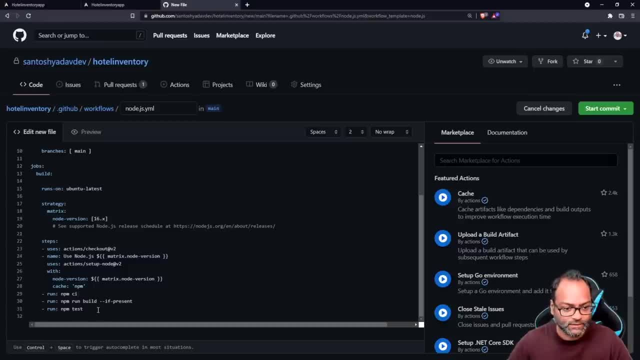 install. And then we are saying that in case the build command is available, just go ahead and build. So we do have the build command, which is build prod. So we'll copy this command and we'll post it. put it here. 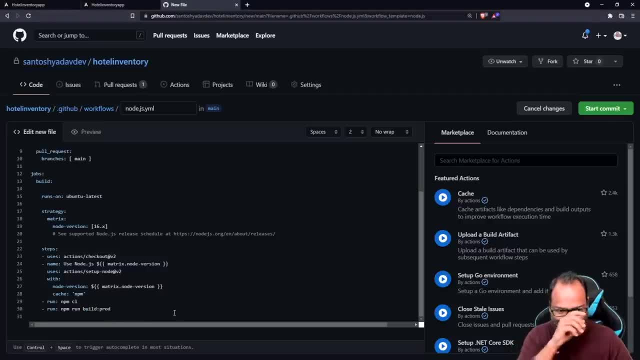 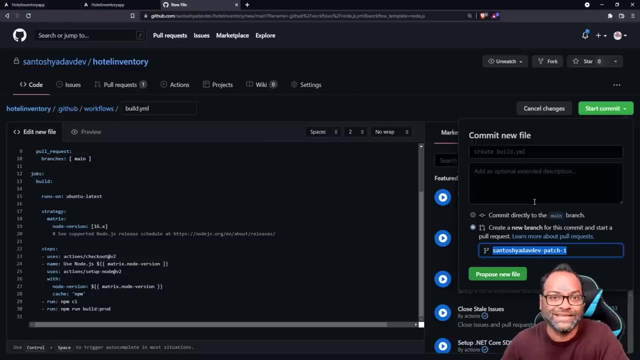 and NPM run build And we'll remove if, if present, because we know that it is available and we'll call it as buildpyml And we'll start a commit. We will create a new branch because we want to see how GitHub actions triggers the changes, right, And we'll say okay. 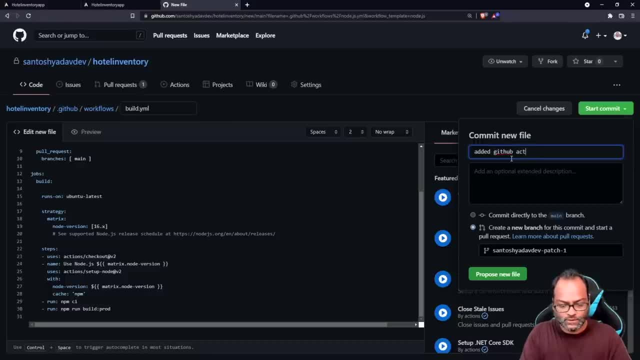 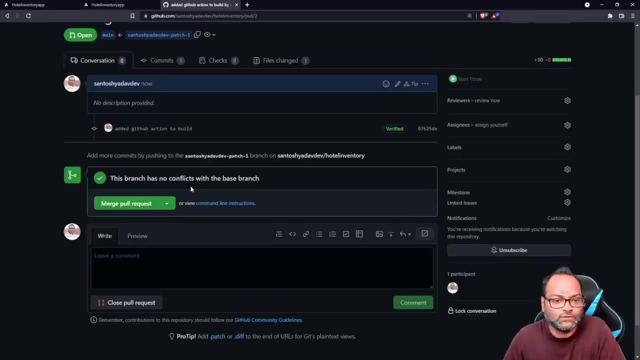 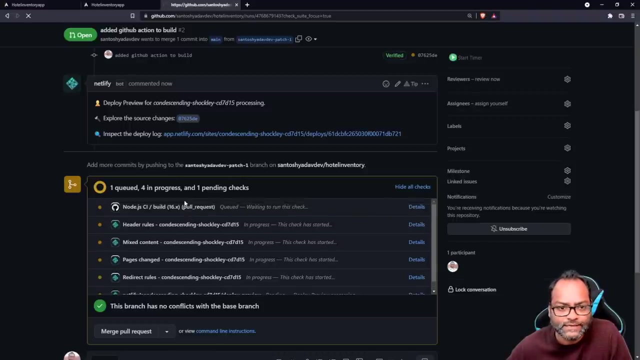 GitHub action to build And let's propose a new file And let's create a pull request. On pull request, it will start building your code right. So here let's go ahead and see. Now you can see there is a new step which is added here- nodejs CI- And you can click on details to see what is. 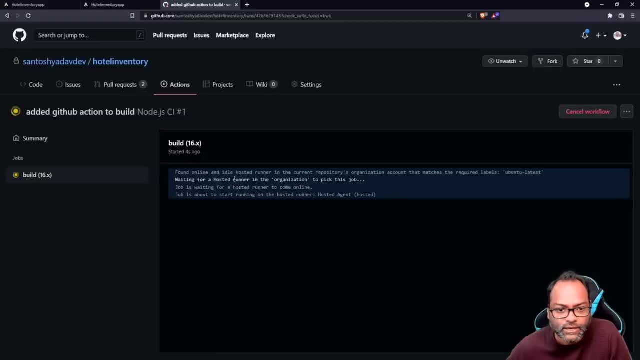 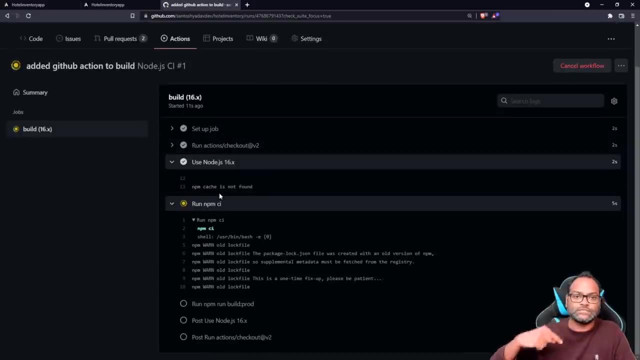 happening here. So you- it started a new job, starting a new job And it is setting up your job And it is executing all the step which we mentioned in that YML file. So you don't have to become like a DevOps expert to do this GitHub action. make it really easy. 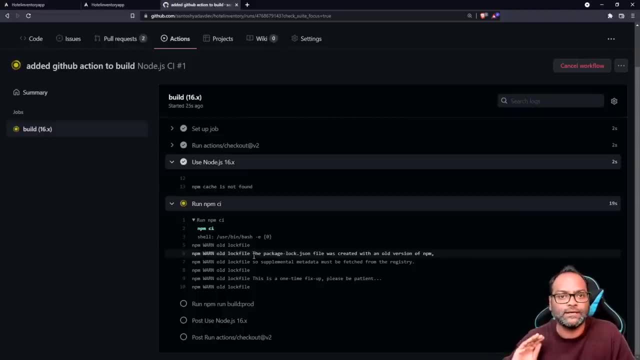 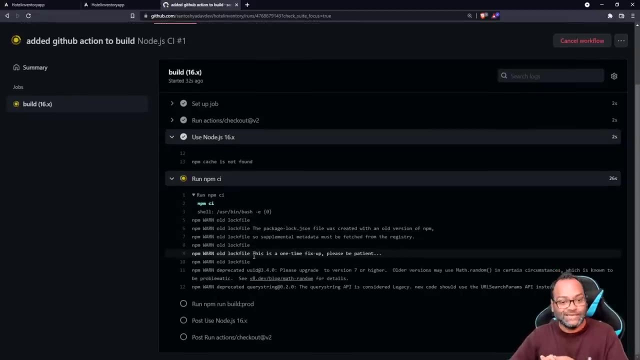 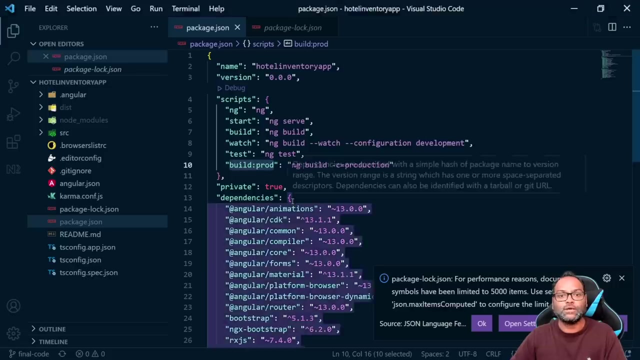 for us. So we just need to choose right template and then give the right commands to execute or build your code base. You can also run your tests on CI So you can verify all the changes before you go ahead and merge your code. Remember, Netlify is good. 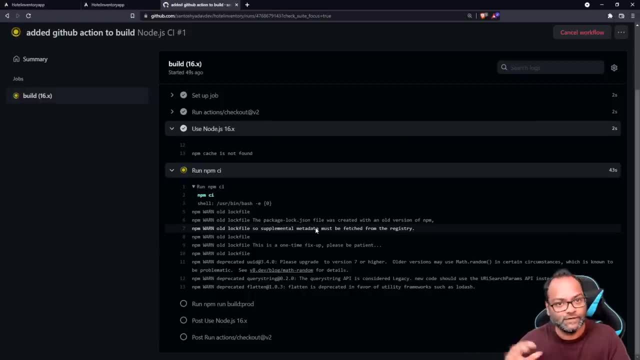 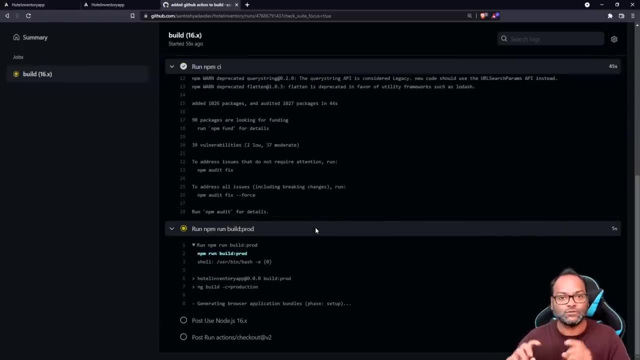 It will check if your build is completed and it will give you a deploy URL. But what in case? we want to do more. we want to run the tests. we want to run the end-to-end tests. So GitHub actions can help you with those. You can just go ahead and give those commands in sequence and it will run.